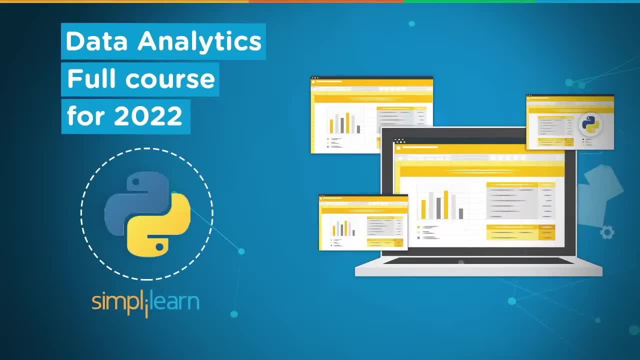 business performances as well as results, and use that information to prepare for the future. That, essentially, is data analytics. So, hey, everyone, welcome to this interesting video tutorial of Data Analytics Full Course 2022 by Simply Learn. This video will help you gain all the necessary skills and knowledge within 12 hours to become a data analyst in 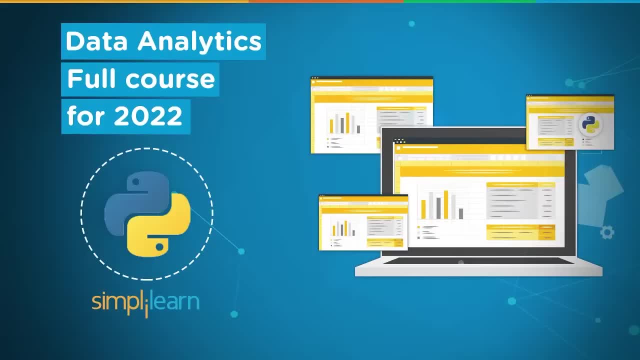 2022.. Our experienced trainers will take you through the course. But before we begin, if you love watching tech videos, subscribe to our channel and hit the bell icon to never miss an update from us. So let's look at the topics we'll be learning in this video. 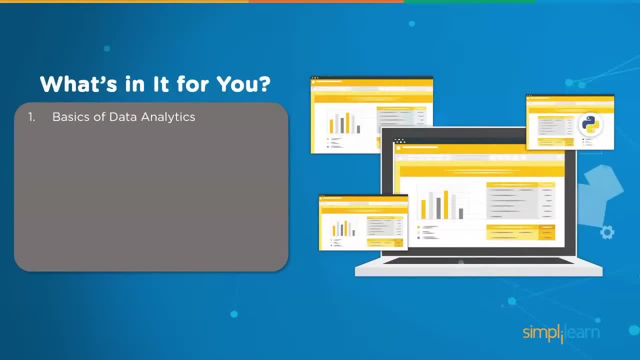 We'll start by understanding the basics of data analytics and learn the top 10 data analyst skills for 2022.. After that, we learn the top 10 data analysis tools, followed by looking at a use case in Python. Next, you'll get an idea of how to manipulate and visualize data using R packages and then 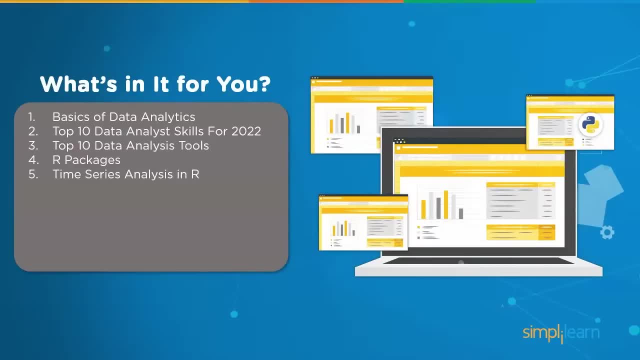 look at time series analysis in R. Then we'll shift our focus to understanding data analytics using Excel pivot tables and learn to create Excel dashboards. Moving further, you'll see some interesting data analytics projects related to Coronavirus, Spotify, World Happiness Report and Hoopla. 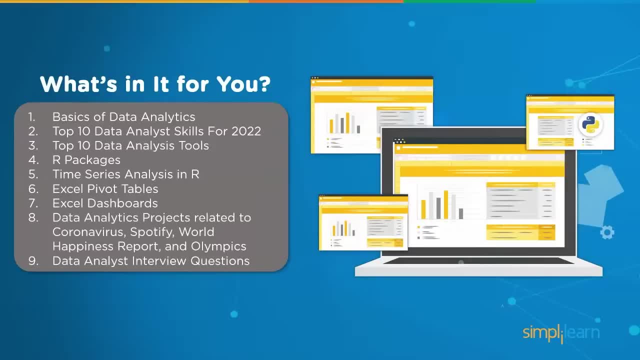 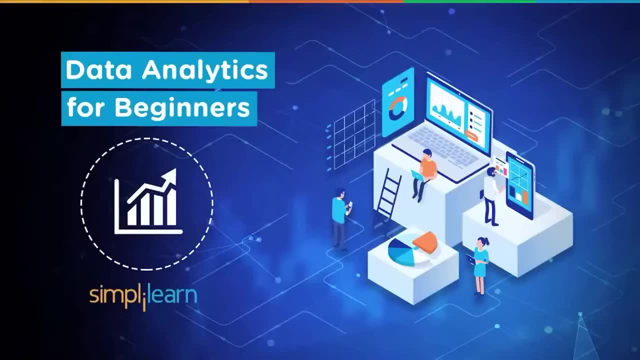 Finally, we'll learn some of the important questions that are asked frequently in data analytics interviews. So let's get started. Hi guys, welcome to another video tutorial by Simply Learn. In today's session, we will look at data analytics for beginners, But before we begin, make sure to subscribe to. 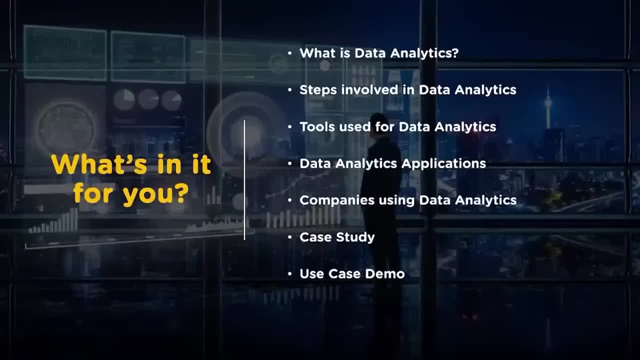 our channel and hit the bell icon to never miss an update. In this video, we will discuss what data analytics is and the need for data analytics. Then we will look at the different ways in which data analytics can be used, followed by the various steps involved in the data analytics process. 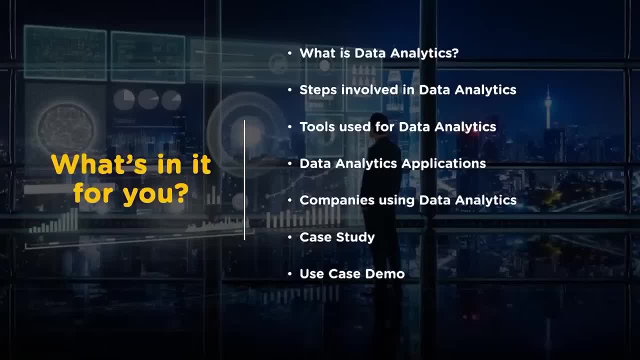 After that, we will get an idea about the different tools used in data analytics and the companies using data analytics. Moving forward, we will see a case study on how Walmart uses data analytics for better customer service And finally, we will perform a regression analysis in R to predict sales based on the 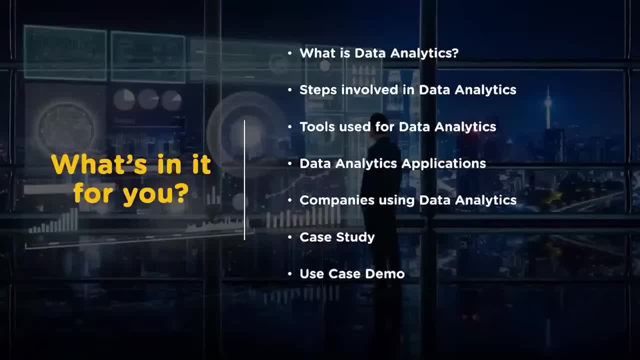 our channel and hit the bell icon to never miss an update. In this video, we will discuss what data analytics is and the need for data analytics. So let's get started. Then we'll look at the different ways in which data analytics can be used. followed. 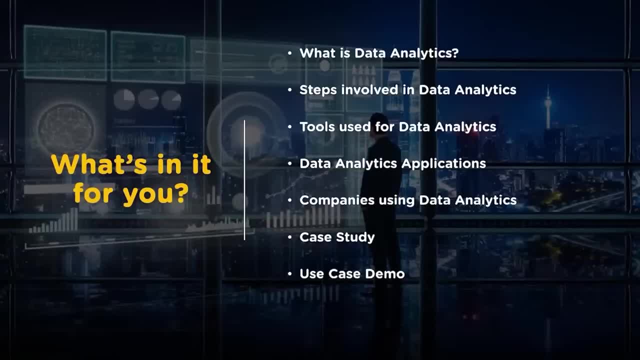 by the various steps involved in the data analytics process. After that, we'll get an idea about the different tools used in data analytics and the companies using data analytics. Moving forward, we'll see a case study on how Walmart uses data analytics for better. 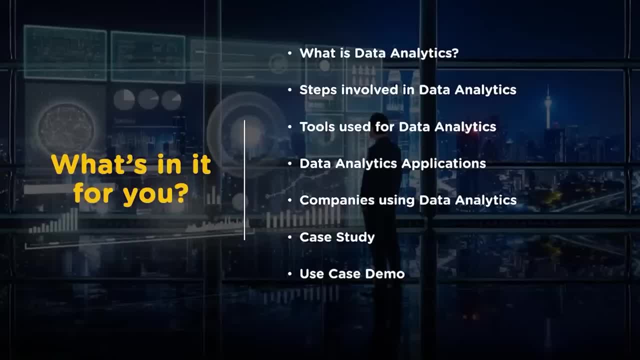 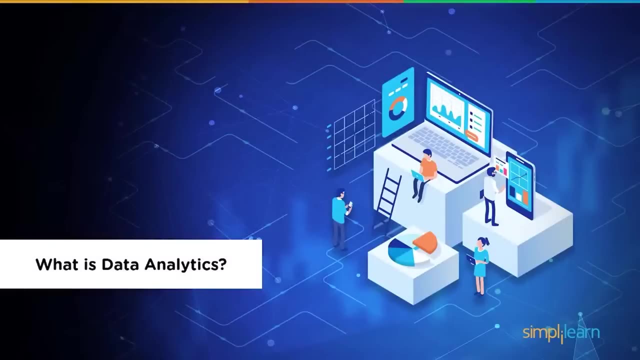 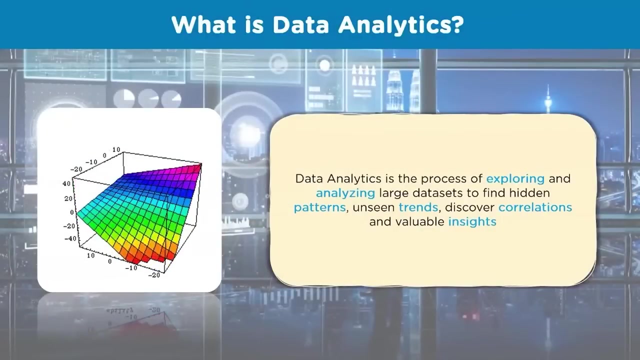 customer service. And finally, we'll perform a regression analysis in R to predict sales based on the advertising data: TV ads, radio ads and newspaper advertisements. So what is data analytics? Companies around the world are generating vast volumes of data every hour. This data 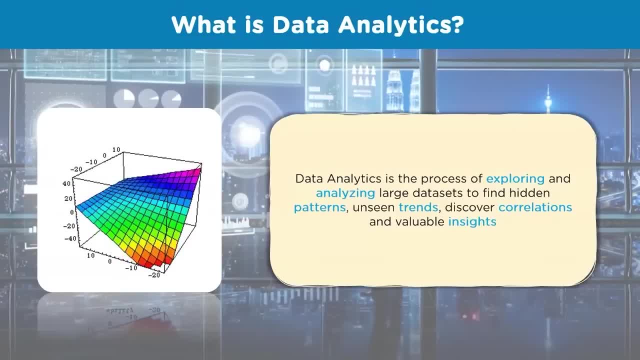 could be in the form of log files, web server and transactional data, as well as various customer related data. Also, data is being generated at a rapid rate from social media websites and applications such as Facebook, Twitter and Google. Companies want to use this data to derive value out of it and make business decisions. 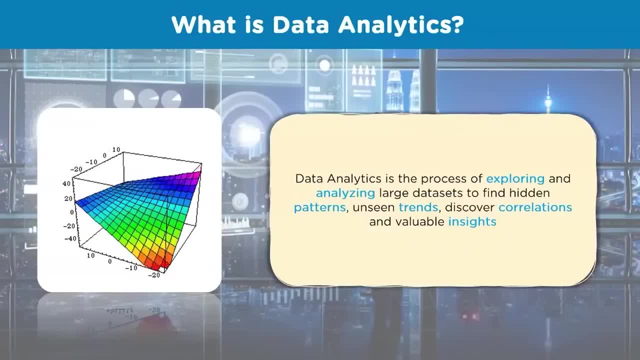 That's where data analytics comes into use. Data analytics is the process of exploring and analyzing large datasets to find hidden patterns, unseen trends, discover correlations and valuable insights to make business predictions. Data analytics improves the speed and efficiency of your business. A few years ago, a business would have gathered information manually performed statistical. 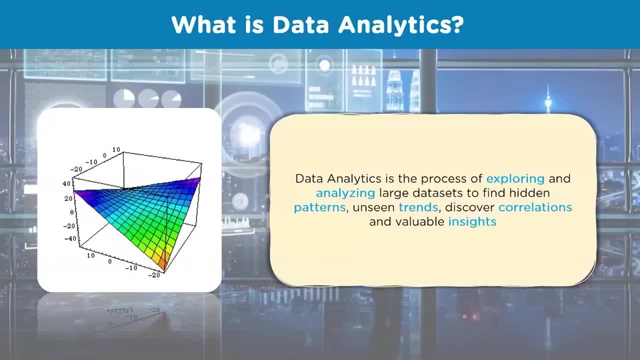 and complex analytics and unearthed information that could be used for future decisions. But today that business can identify insights on the fly for immediate decisions. Most organizations have big data and many understand the need to harness that data and extract value out of it. 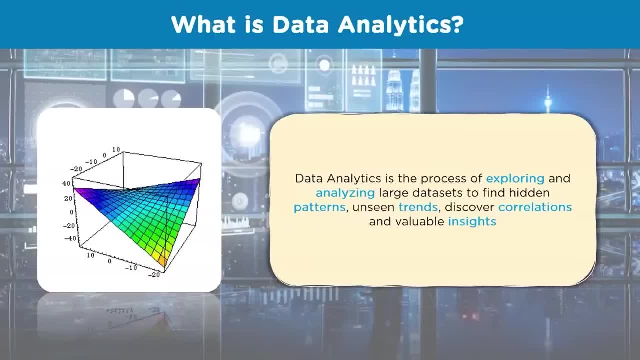 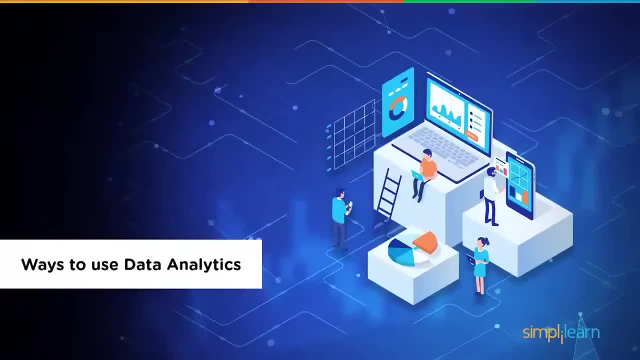 So they use a lot of modern tools and technologies to perform data analytics. So they use a lot of modern tools and technologies to perform data analytics. Some of the tools I will discuss in detail later in this tutorial. Now that we have looked at what data analytics really is, let us understand the ways in which 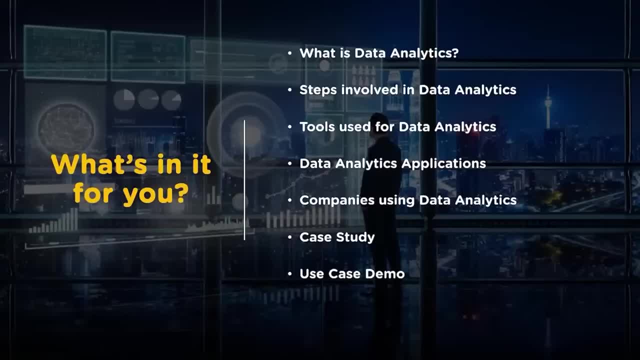 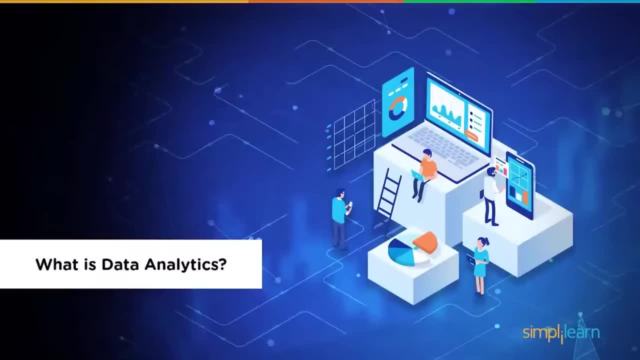 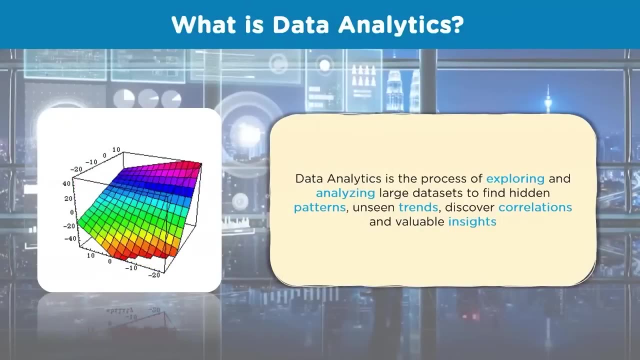 advertising expenditure from 3 minutes, So let's get started. So what is data? analytics? Companies around the world are generating vast volumes of data every hour. This data could be in the form of log files, web server and transactional data, as well as various 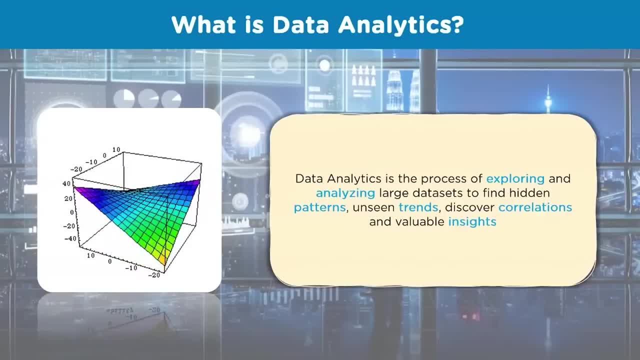 customer-related data Also, data is being generated at a rapid rate from social media websites and applications such as Facebook and Twitter. Companies want to use this data to derive value out of it and make business decisions. That's where data analytics comes into use. 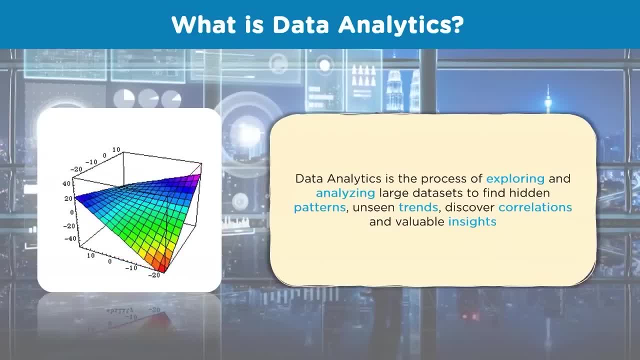 Data analytics is the process of exploring and analyzing large datasets to find hidden patterns, unseen trends, discover correlations and valuable insights to make business predictions. Data analytics improves the speed and efficiency of your business. Data analytics improves the speed and efficiency of your business. 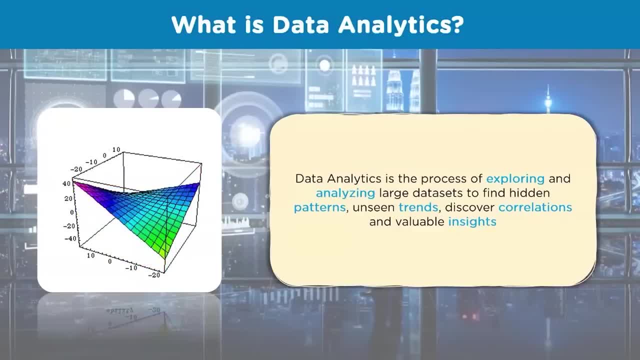 Data analytics improves the speed and efficiency of your business. A few years ago, a business would have gathered information manually, performed statistical and complex analytics and unearthed information that could be used for future decisions. But today, that business can identify insights on the fly for immediate decisions. 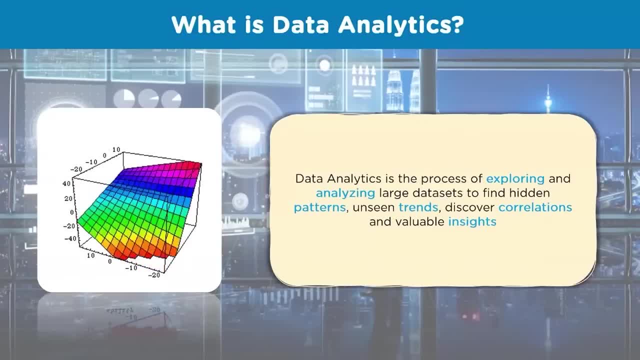 Most organizations have big data and many understand the need to harness that data and extract value out of it. So they use a lot of modern tools and technologies to produce data analytics and technologies to perform data analytics. Some of the tools I will discuss in detail. 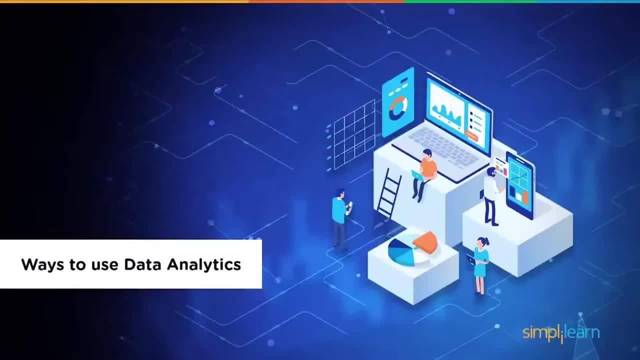 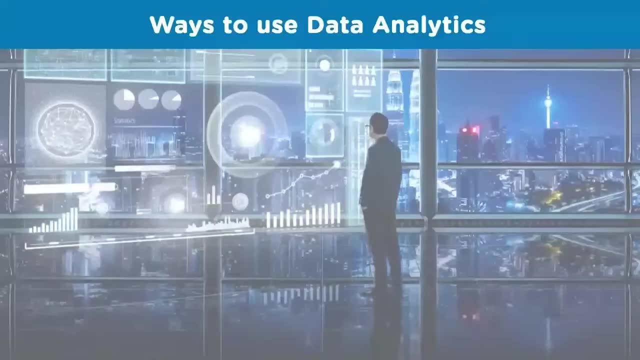 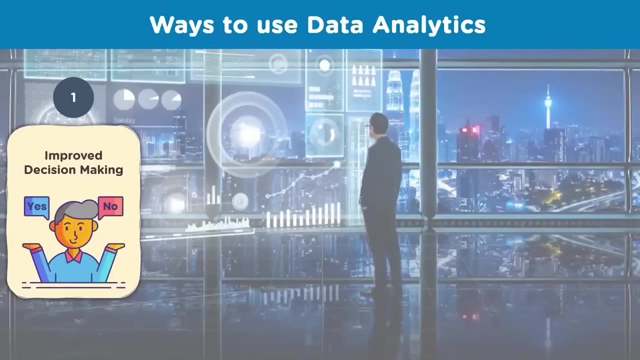 later in this tutorial, Now that we have looked at what data analytics really is, let us understand the ways in which you can use data analytics. First is improved decision making. Data analytics eliminates a lot of guesswork and manual tasks from choosing the right content, planning marketing campaigns and developing products. 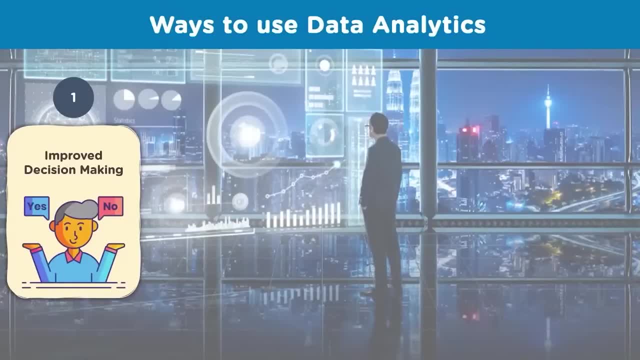 Organizations can use the insights they gain from data analytics to make informed decisions leading to better outcomes and customer satisfaction. It gives you a 360 degree view of your customers, which helps you understand the behavior, completely enabling you to better meet their needs. Second is better customer service. Data analytics provides you with more accurate 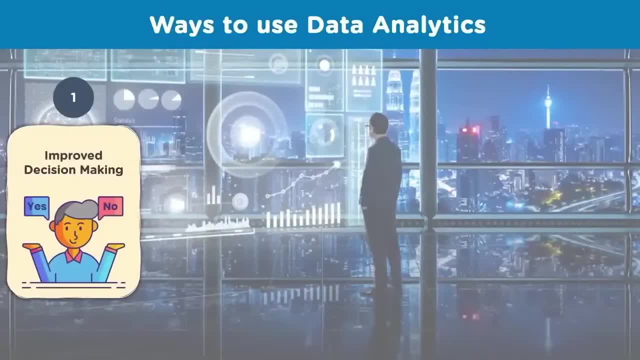 you can use data analytics First is improved decision making. Data analytics eliminates a lot of guesswork and manual tasks from choosing the right content, planning marketing campaigns and developing products. Organizations can use the insights they gain from data analytics to make decisions. 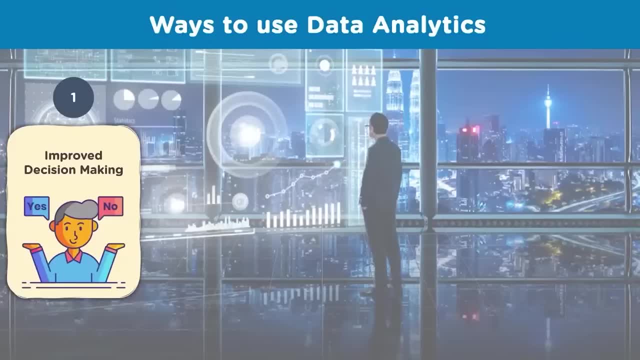 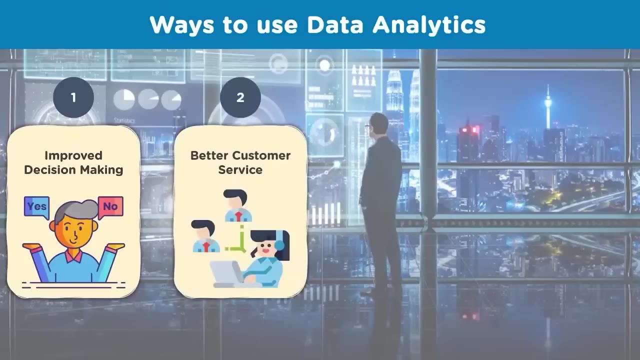 They can use data analytics to make informed decisions leading to better outcomes and customer satisfaction. It gives you a 360 degree view of your customers, which helps you understand their behavior completely, enabling you to better meet their needs. Second is better customer service. 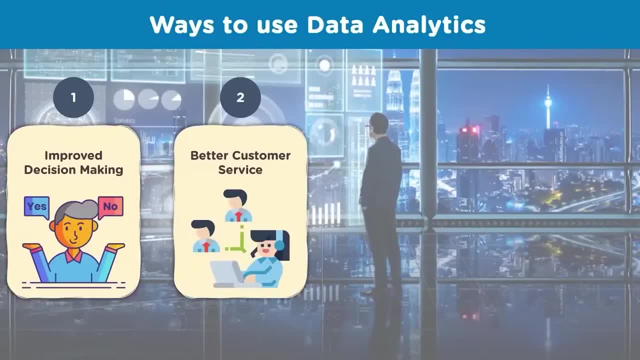 Data analytics provides you with more accurate insights of your customers, allowing you to tailor customer service to their needs, provide more personalization and build stronger relationships with them. Your data can reveal information about your customers' communication preferences, their interests, their concerns and more. 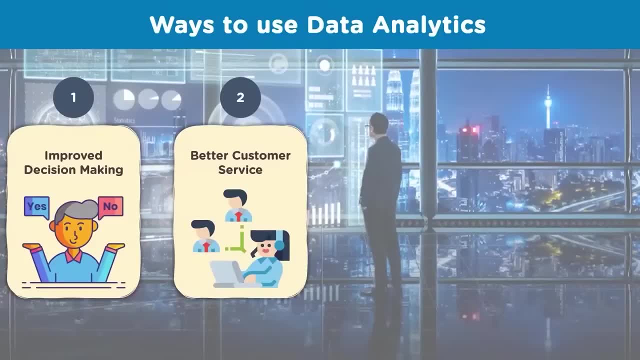 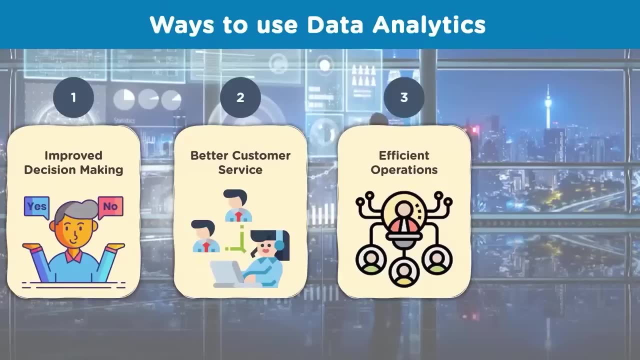 It helps you give better recommendations for products and services. Next is efficient operations. Data analytics can help you streamline your processes, save money and boost production. When you have an improved understanding of what your audience wants, you waste less time in creating ads and content that don't match your audience's expectations. 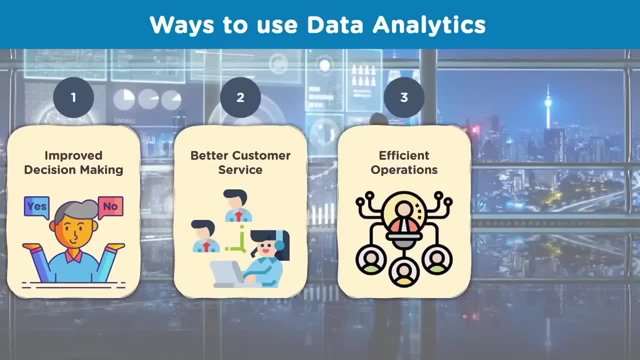 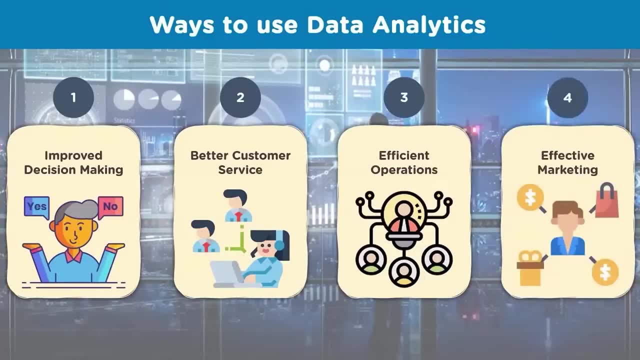 This helps you optimize your campaigns, create better content strategies and hence improve results. And finally, we have effective marketing. When you understand your audience better, you can market to them more effectively. Data analytics also gives you useful insights into how your campaigns are performing, so 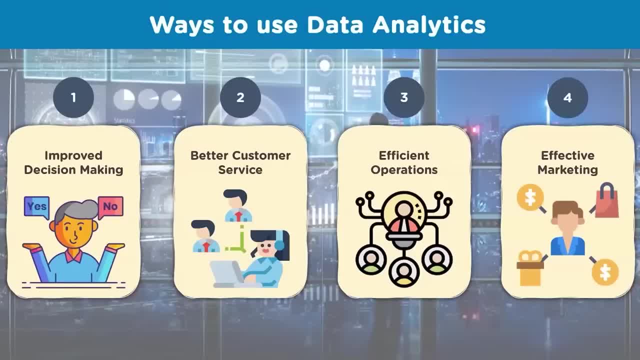 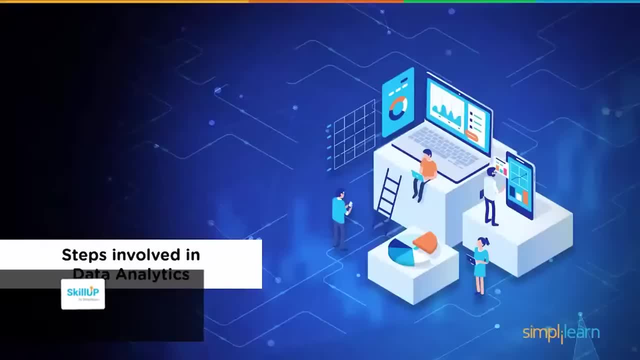 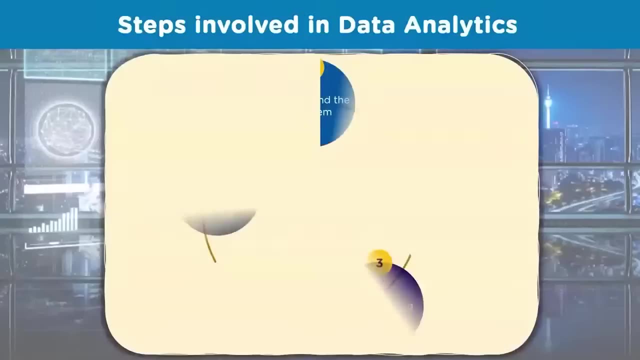 that you can fine-tune them for optimal outcomes. You also find out the probable customers who are the most likely to interact with a campaign and convert into leads. Now let's discuss the various steps involved in the data analytics process. As you can see on the screen, there are five process steps. 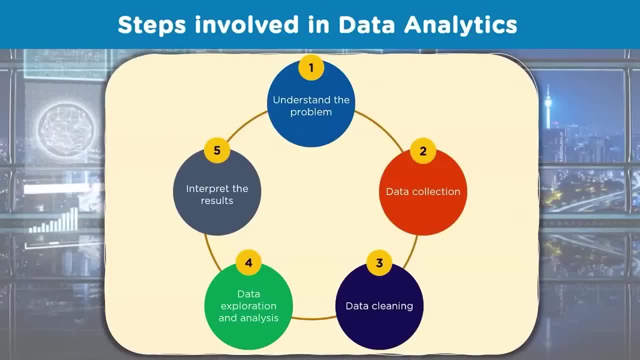 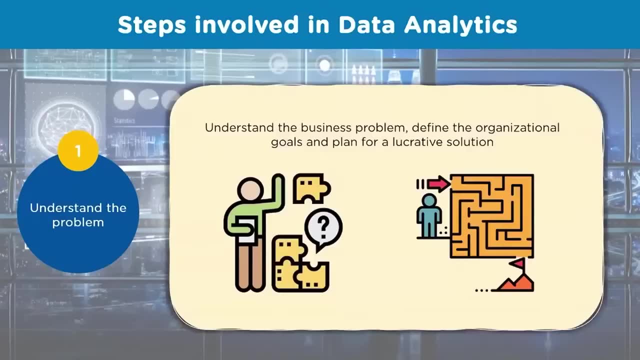 Now let me make you understand each of these one by one. So the first step is to understand the problem. Before starting with the analysis, you need to understand the business problem and define your goals. Asking questions at the outlet is vital, because this would address issues such as: how can 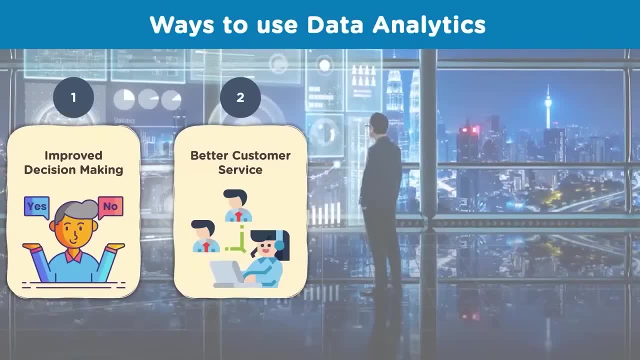 insights of your customers, allowing you to tailor customer service to their needs and provide more personalization and build stronger relationships with them. Your data can reveal information about your customers communication preferences, their interests, their concerns and more. It helps you give better recommendations for products and. 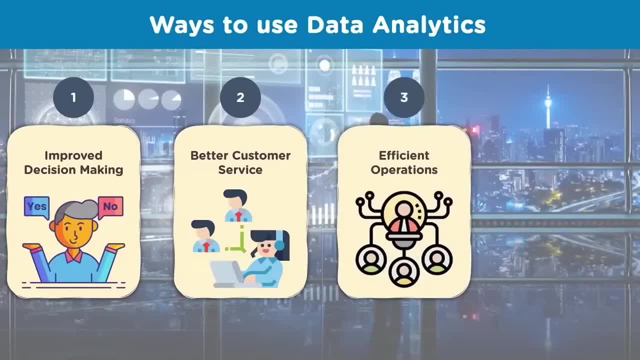 services. Next is efficient operations. Data analytics can help you streamline your processes, save money and boost production. When you have an improved understanding of what your audience wants, you waste less time in creating ads and content that don't match your audience interests. 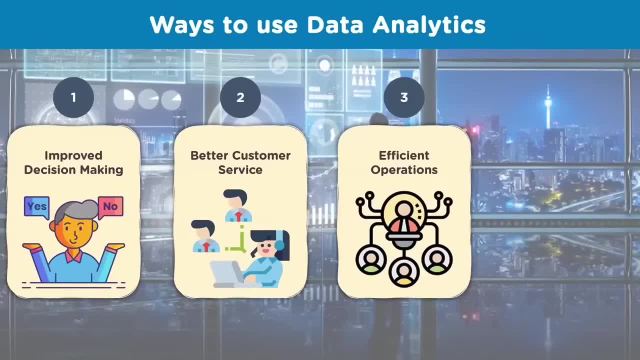 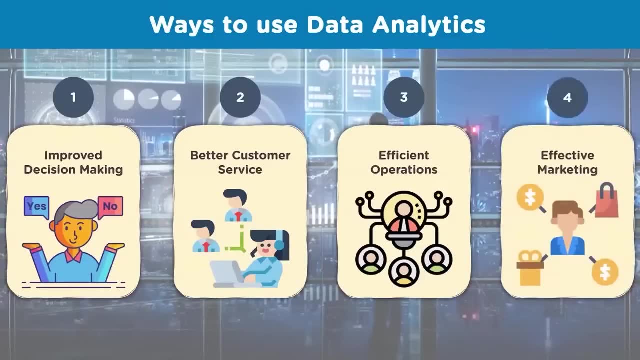 This helps you optimize your campaigns, create better content strategies and hence improve results. And finally, we have effective marketing. When you understand your audience better, you can market to them more effectively. Data analytics also gives you useful insights into how your campaigns are performing so that you can fine tune them for optimal outcomes. You also find 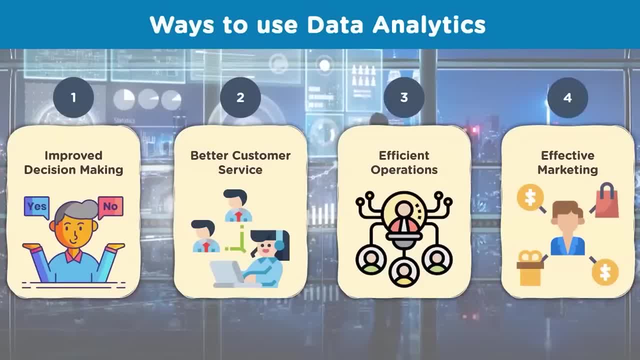 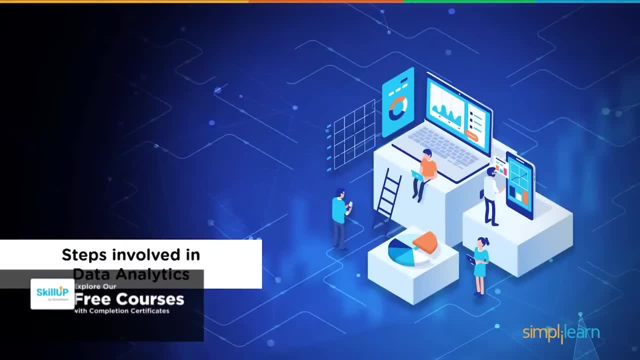 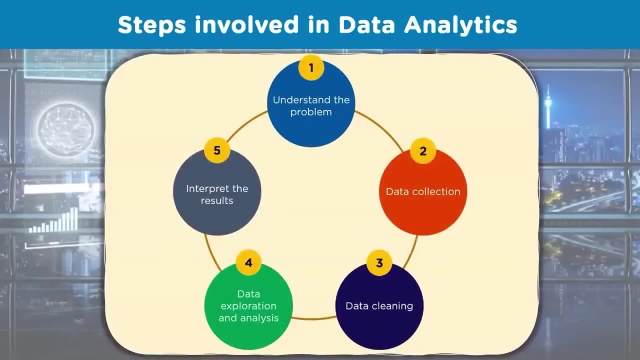 ways with which you can showcase your audience's longest lasting success. dentuities He bubble customers who are the most likely to interact with a campaign and convert into leads. Now let's discuss the various steps involved in the data analytics process. As you can see on the screen, there are five process steps. 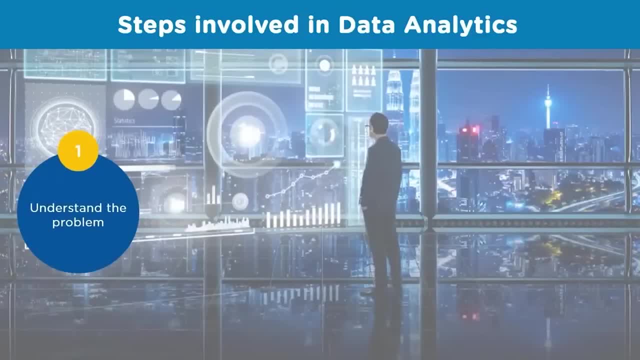 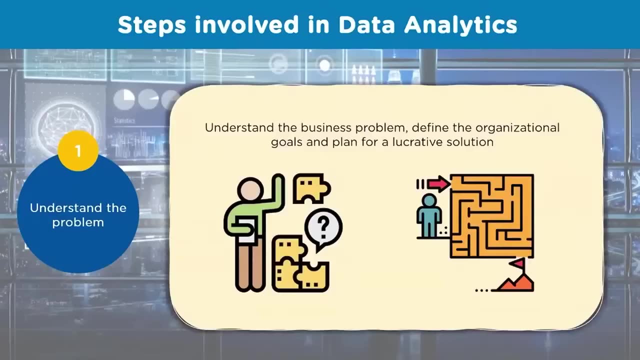 Now let me make you understand each of this one by one. So the first step is to understand the problems. you need to understand the business problem and define your goals. asking questions at the outlet is vital because this would address issues such as: how can we reduce production costs without sacrificing quality? what are some of the 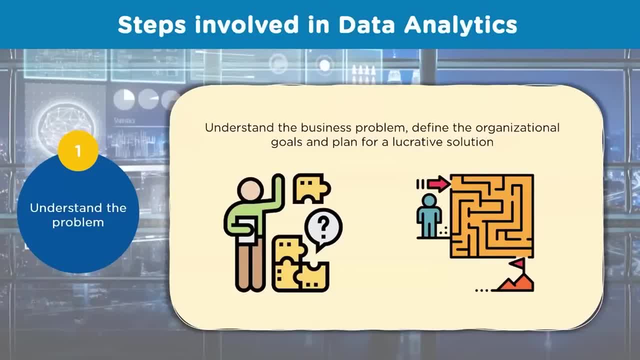 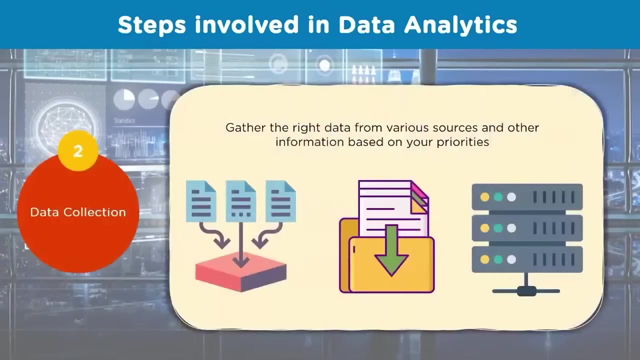 ways to increase sales opportunities with our current resources? do customers view our brand in a favorable way? answers to these questions will help you build a clear roadmap with lucrative solutions. also try to find out the key performance indicators and consider the matrix to track along the way. the second step in the process is data collection after you have finalized your 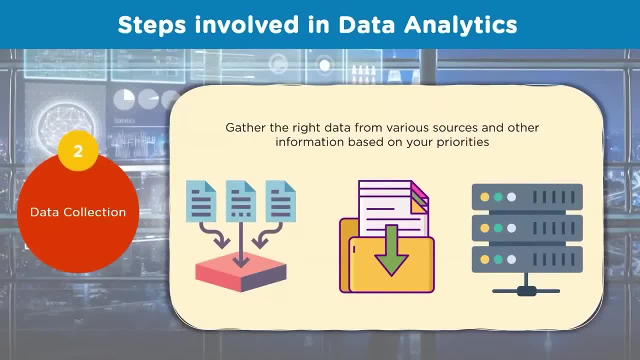 goals. it's time to start looking for your data. data collection is the process of gathering information on targeted variables identified as data requirements. the emphasis is on ensuring accurate and right data is collected. data collection starts with primary sources, which are also known as internal sources. this is typically structured data gathered from CRM software ERP. 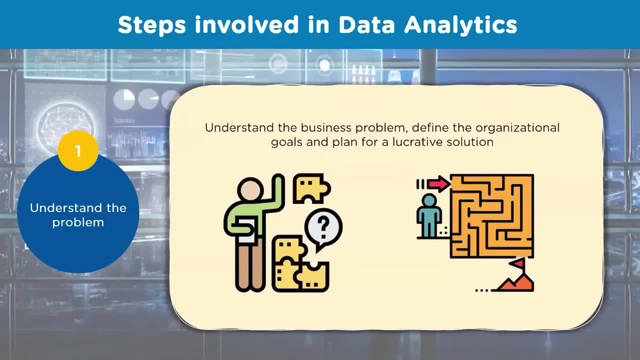 we reduce production costs without sacrificing quality. What are some of the ways to increase sales opportunities with our current resources? Do customers view your brand in a favorable way? Answers to these questions will help you build a clear roadmap with lucrative solutions. Also, try to find out the key performance indicators and consider the matrix to track. 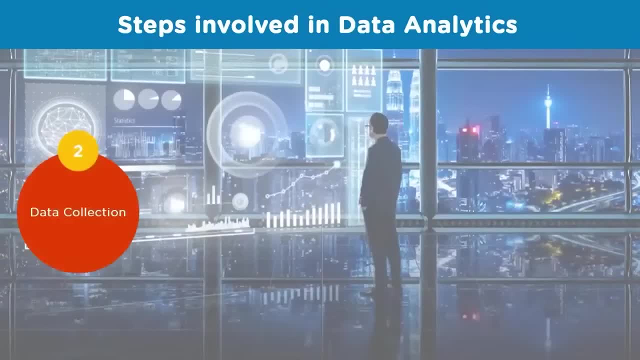 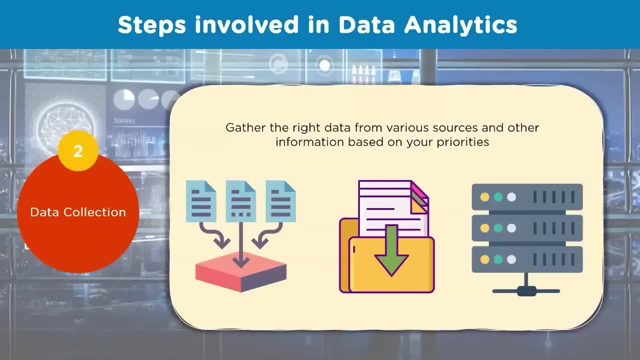 along the way. The second step in the process is data collection. After you have finalized your goals, it's time to start looking for your data. Data collection is the process of gathering information on targeted variables identified as data requirements. The emphasis is on ensuring accurate and right data is collected. 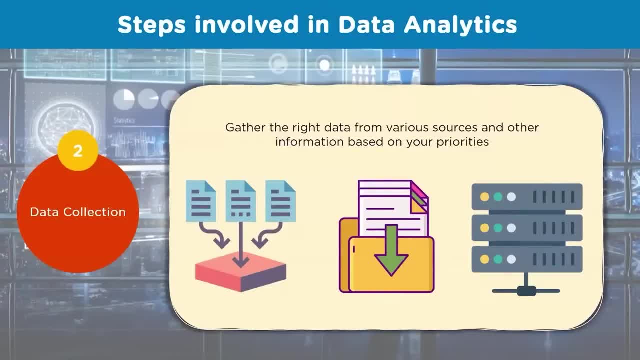 Data collection starts with primary sources, which are also known as internal sources. This is typically structured data gathered from CRM software, ERP systems, marketing automation tools and others. These sources contain information about customers, finances, gaps in sales, etc. Under external sources, you have both structured and unstructured data. 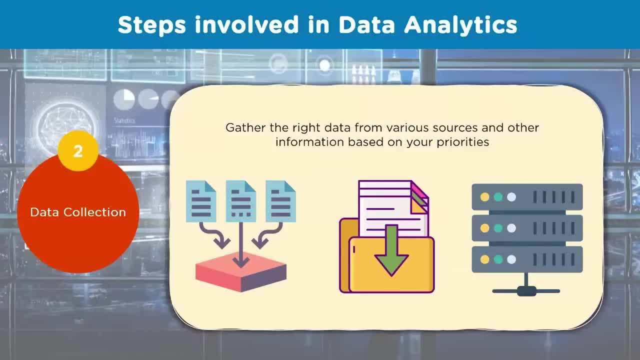 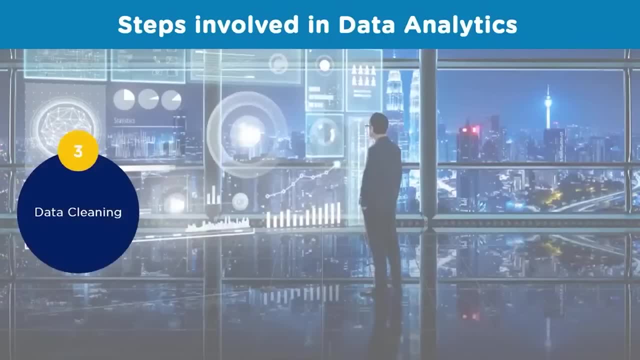 So, if you are looking to perform a sentiment analysis towards your brand, you would gather data from various review websites or social media apps. The next step is to clean the data. The data which is collected is then stored in a database. Data collection is the process of collecting data from various review websites or social 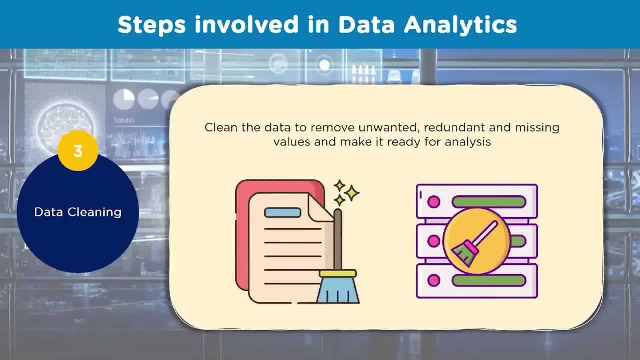 media apps. The data which is collected from various sources is highly likely to contain incomplete, duplicate and missing values, So you need to clean these unwanted, redundant data to make it ready for analysis. So, to generate accurate results, analytics professionals must identify duplicate and 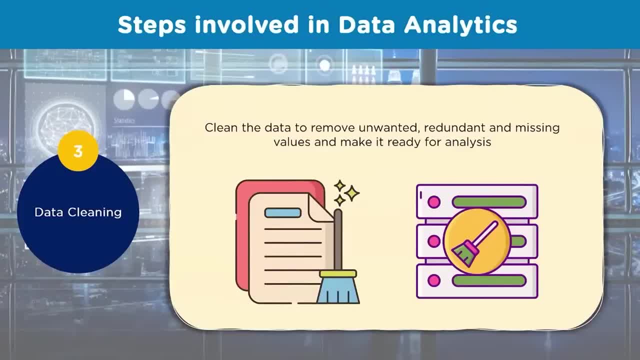 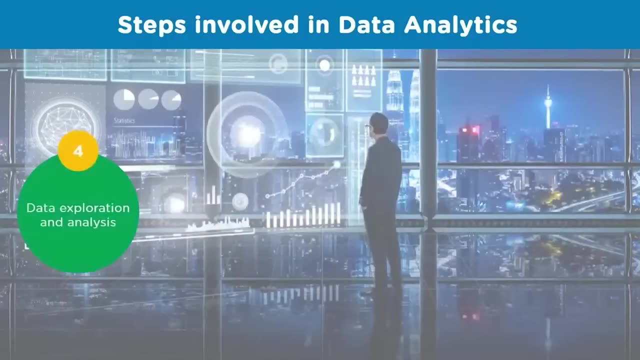 anomalous data and other inconsistencies that could skew the analysis. According to a report, 60% of data scientists say most of the time is spent cleaning the data, while 57% of data scientists say it's their least energy-consuming task. Now the fourth step in the process is data exploration and analysis. 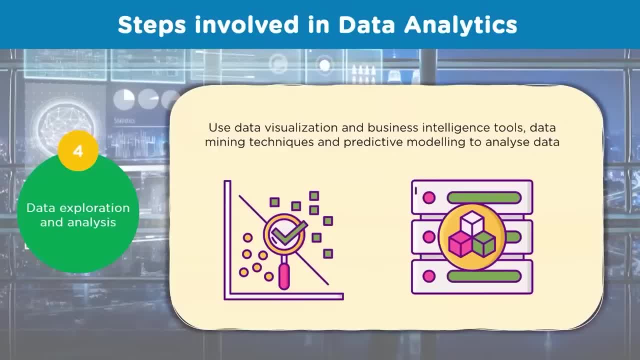 Once data is cleaned and ready, you can go ahead and explore the data using data visualization and business intelligence tools. You can also use various data mining and predictive modeling techniques to analyze the data and build models. You can use different supervised and unsupervised algorithms, such as linear regression, logistic. 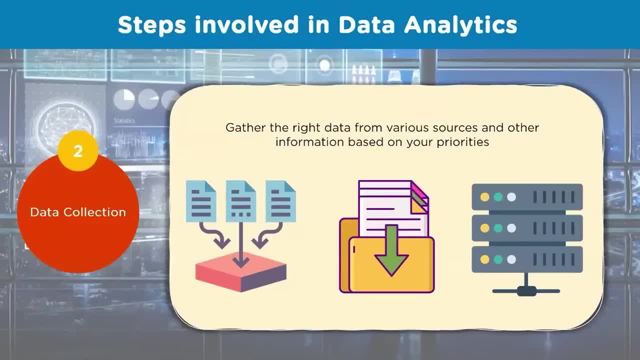 systems, marketing automation tools and others. these sources contain information about customers, finances, gaps in sales, etc. under external sources, you have both structured and unstructured data. so if you are looking to perform a sentiment analysis towards your brand, you would gather data from various review websites or social media apps. 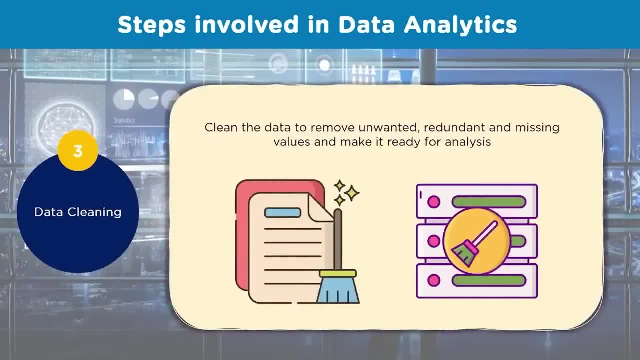 the next step is to clean the data. the data, which is collected from various sources, is highly likely to contain incomplete, duplicate and missing values, so you need to clean these unwanted, redundant data to make it ready for analysis. so, to generate accurate results, analytics professionals must identify duplicate and anomalous data and other inconsistencies that could skew the 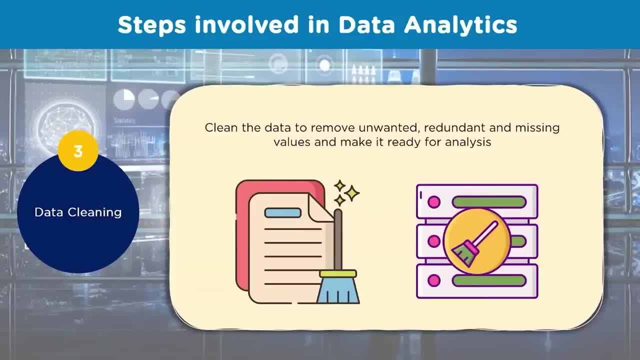 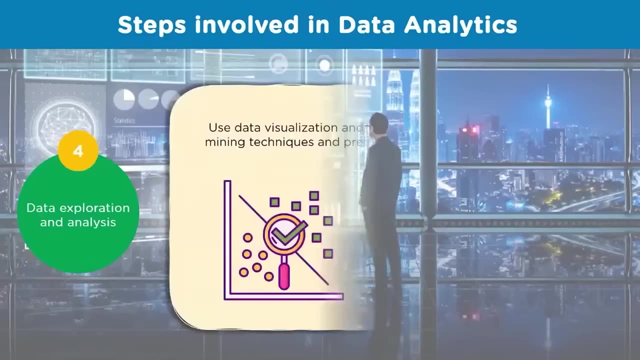 analysis. according to a report, 60% of data scientists say most of the time is cleaning the data, while 57% of data scientists say it's their least enjoyable task. now the fourth step in the process is data exploration and analysis. once data is cleaned and ready, you can go ahead and explore the data. 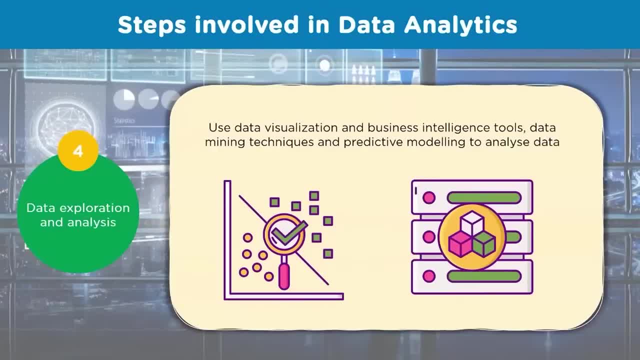 using data visualization and business intelligence tools. you can also use various data mining and predictive modeling techniques to analyze the data and build models. you can use different supervising and unsupervised algorithms, such as linear regression, logistic regression, decision tree, KNN, k-means, clustering and lots more, to build prediction models for. 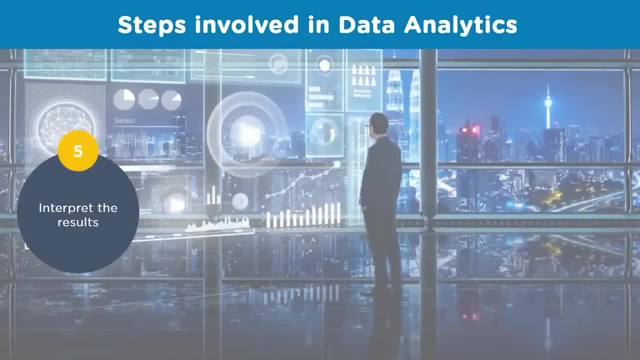 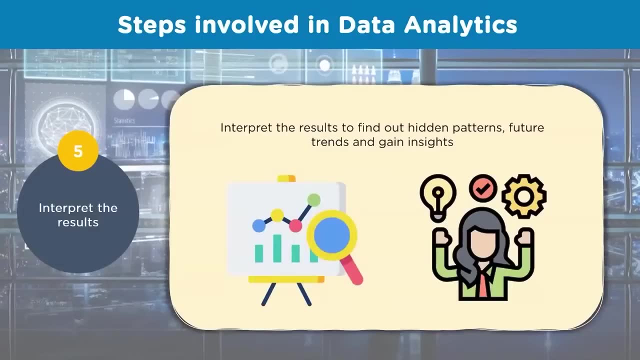 making business decisions, and the final step is to interpret the results. this part is important because it's how a business will gain actual value from the previous four steps. interpreting the results will help you find unseen trends and patterns in the data and gain actual value from the previous four steps. 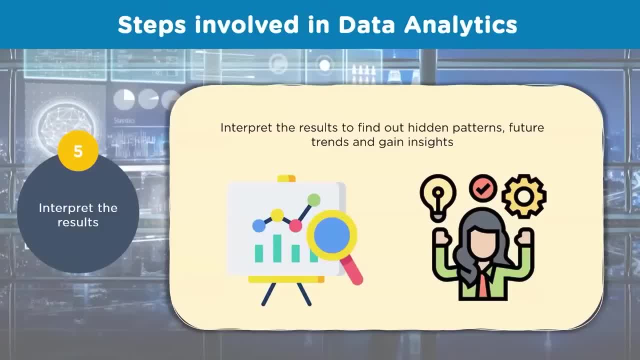 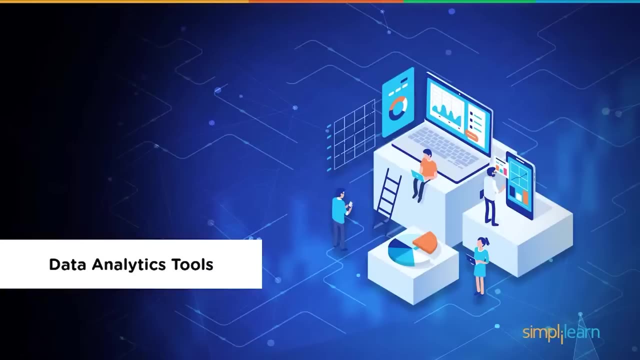 insights. you can have a validation check if the results are answering your questions. these results can be shown to your clients and stakeholders for better understanding and business collaboration. now that we have looked at the various steps involved in data analytics, let's now see the different tools that can be. 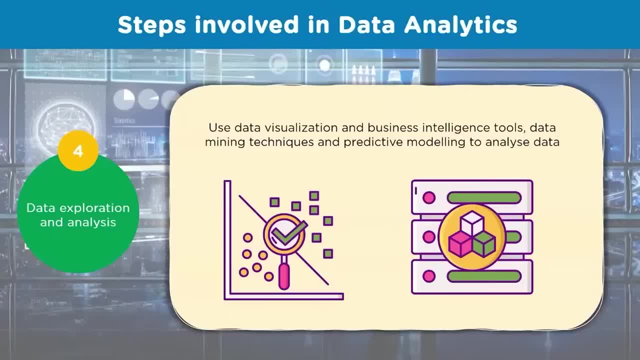 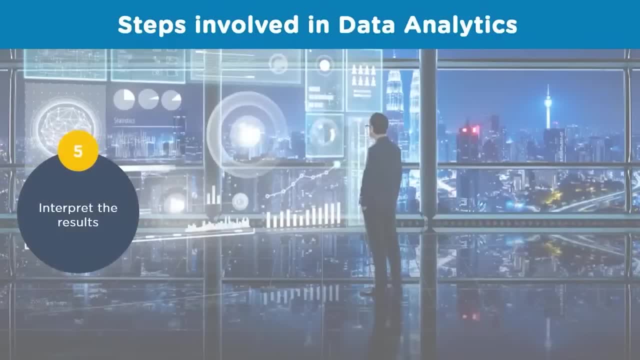 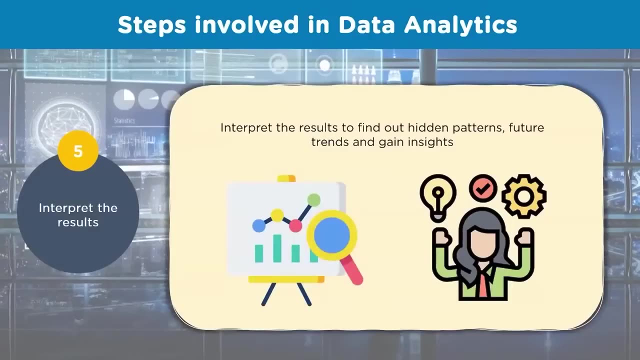 regression, data analysis, etc. Decision tree, KNN, k-means, clustering and lots more to build prediction models for making business decisions, And the final step is to interpret the results. This part is important because it's how a business will gain actual value from the previous. 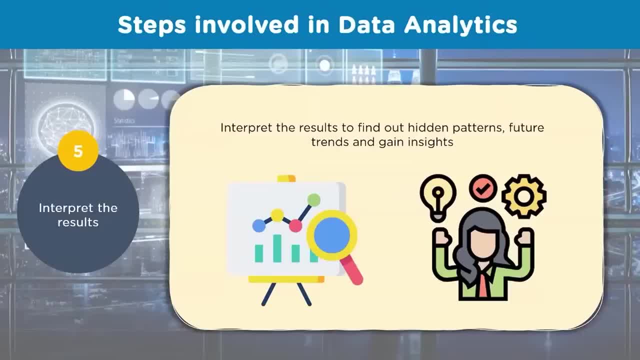 4 steps. Interpreting the results will help you find unseen trends and patterns in the data and gain insights. You can have a validation check if the results are answering your questions. We can also analyze data analysis for the data analysis your questions. These results can be shown to your clients and stakeholders. 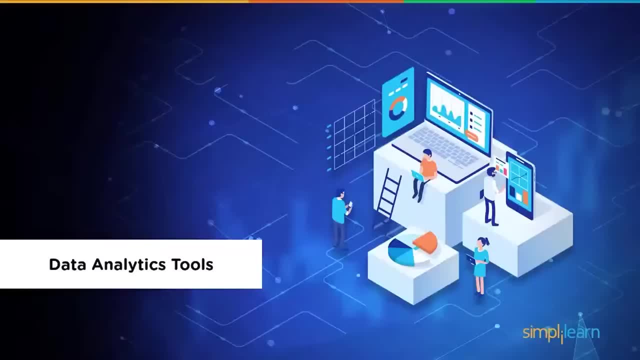 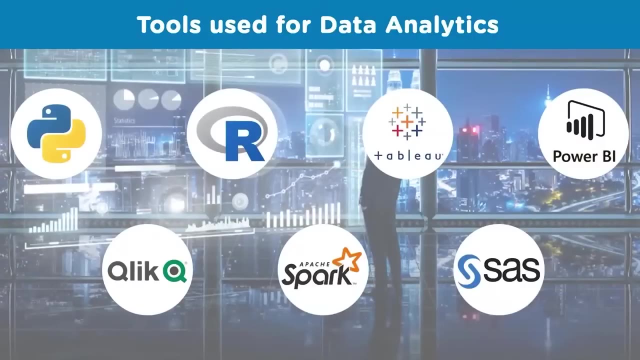 for better understanding and business collaboration. Now that we have looked at the various steps involved in data analytics, let's now see the different tools that can be used to perform the above steps. So, as you can see, we have seven tools, including a few programming languages. 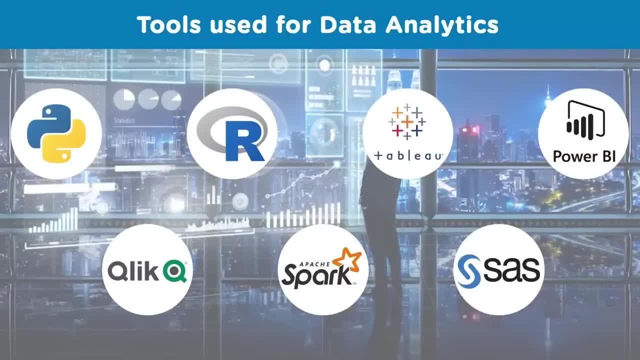 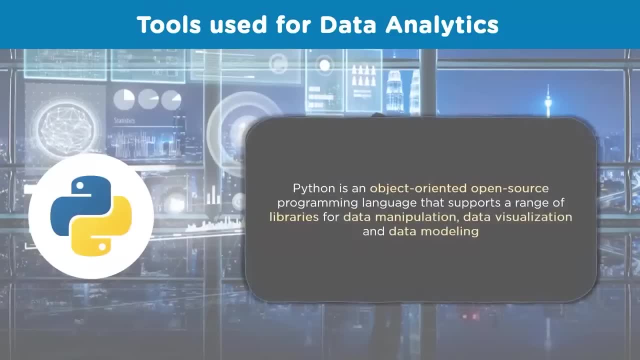 that will help you perform analytics better. Now let's discuss them one by one. First, we have Python. Python is an object-oriented, open-source programming language that supports a range of libraries for data manipulation, data visualization and data modeling. Python programmers have developed tons of free 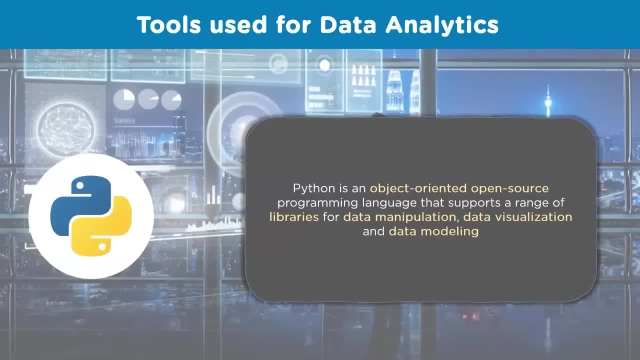 and open-source libraries that you can use. You can find many of them via the Python package index, which is pypi, the repository of Python software. Python provides the default package installer called pip or p-i-p. Python has libraries such as numpy for numerical computation of data, pandas to 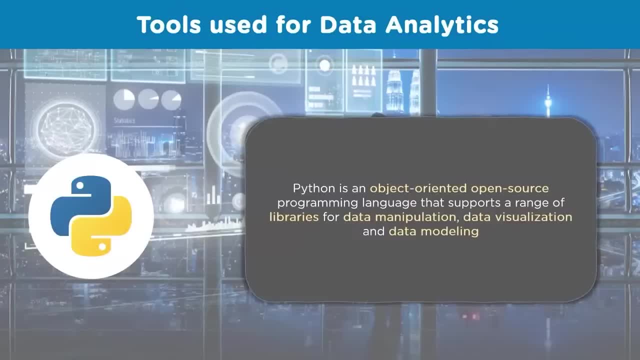 manipulate data on numerical tables and time series. Then you have scipy for technical and scientific computations. It also provides scikit-learn, which is a machine learning library for creating classification, regression and clustering algorithms. and finally, it also has pytorch and tensorflow for deep learning. 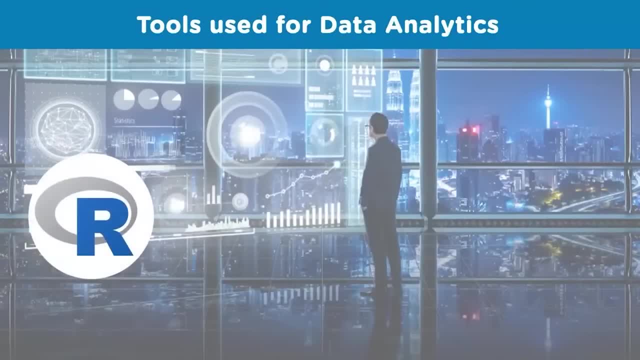 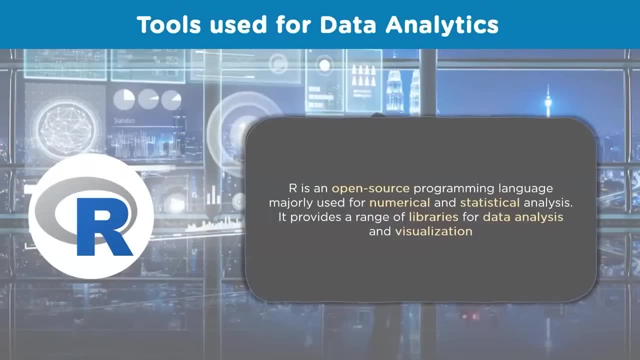 Up next we have R. R is an open-source programming language majorly used for numerical and statistical analysis. It provides a range of libraries for data analysis and visualization. Some of these libraries are ggplot, tidiverse, plotly, dplyr and carrot. Then we have tableau. Tableau is a 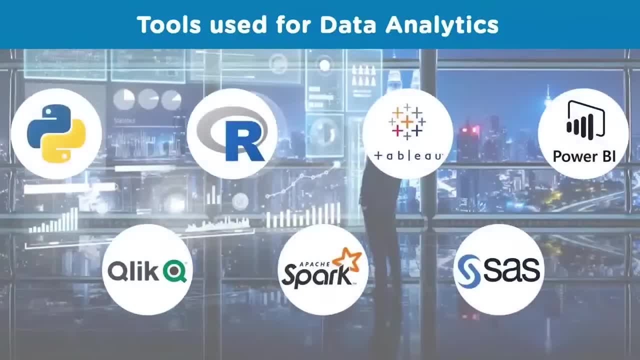 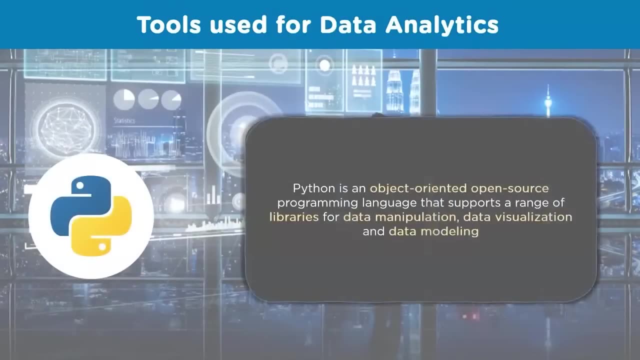 used to perform the above steps. so, as you can see, we have seven tools, including a few programming languages that will help you perform analytics better. now let's go ahead and start the analysis. now let's go ahead and start the analysis. let's discuss them one by one. first, we have Python. 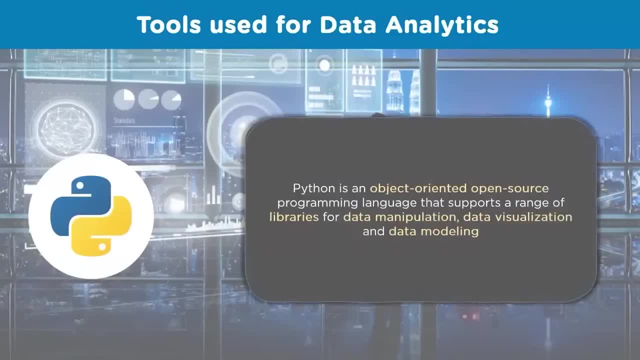 Python is an object-oriented open source programming language that supports a range of libraries for data manipulation, data visualization and data modeling. Python programmers have developed tons of free and open source libraries that you can use. you can find many of them via the Python package index, which is: 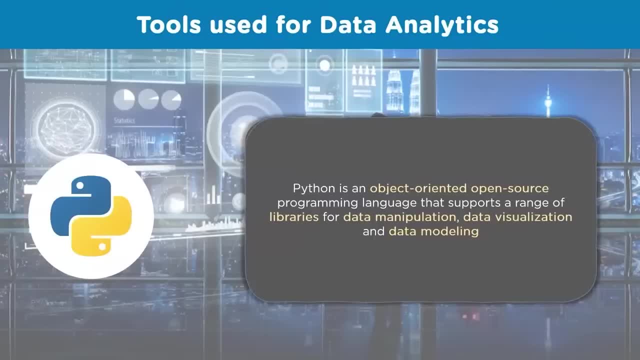 pypi, the repository of Python software. Python provides the default package installer called pip or pip. python has libraries such as numpy for numerical computation of data, pandas to manipulate data on numerical tables and time series. then you have scipy for technical and scientific computations. it also provides scikit-learn, which is a machine learning library for creating classification. 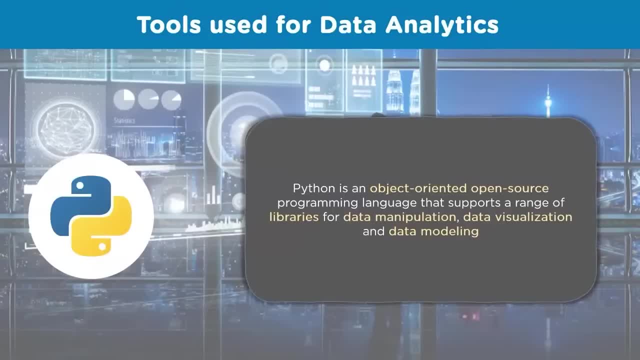 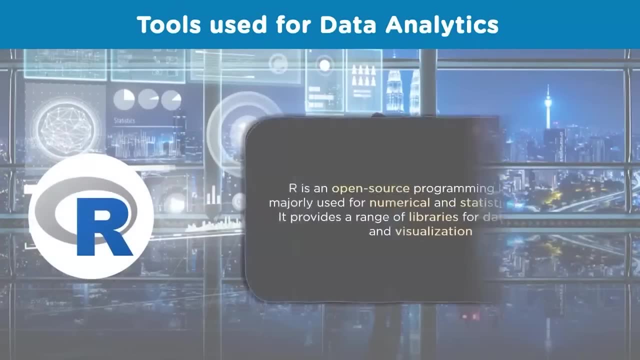 regression and clustering algorithms. and finally, it also has pytorch and tensorflow for deep learning. up next we have R. R is an open source programming language majorly used for numerical and statistical analysis. it provides a range of libraries for data analysis and visualization. some of these libraries are ggplot, tidyverse, plotly, dplyr and. 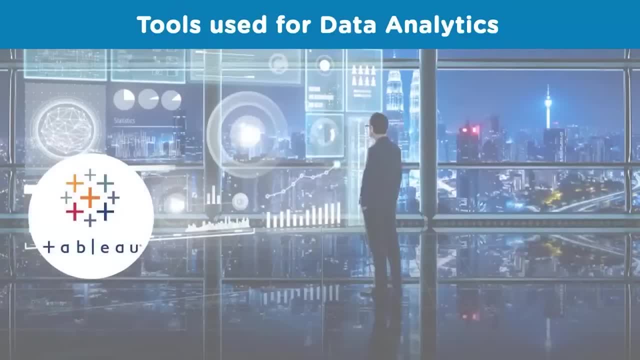 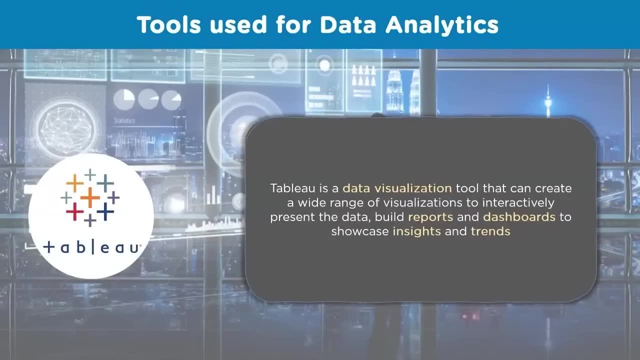 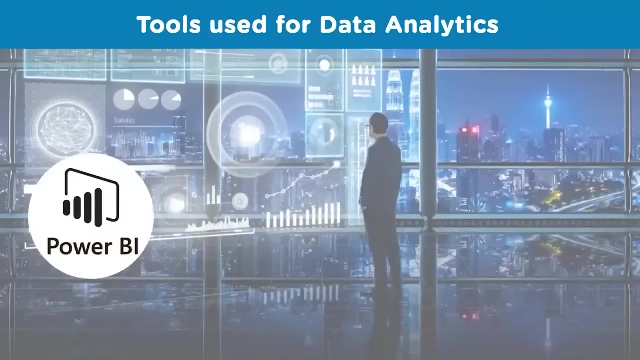 carrot. then we have tableau. tableau is a popular data visualization and analytics tools that helps you create a range of visualizations to interactively present the data, build reports and dashboards to showcase insights and trends. it can connect with multiple data sources and give hidden business insights and patterns. then we have a competitor of tableau, which is 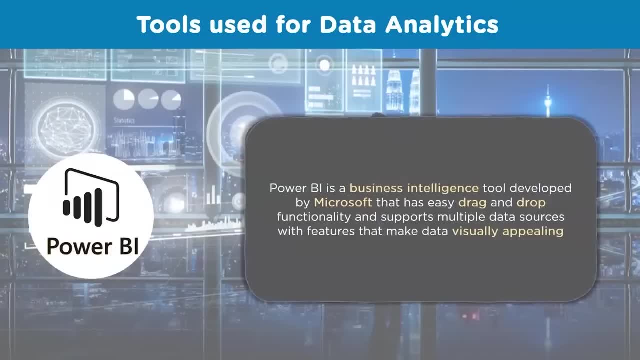 power bi. power bi is a business intelligence tool developed by Microsoft that has an easy drag-and-draw functionality and supports multiple data sources with features that make data visually appealing, power bi supports features that help you ask questions to your data and get immediate insights. you can also forecast your data for 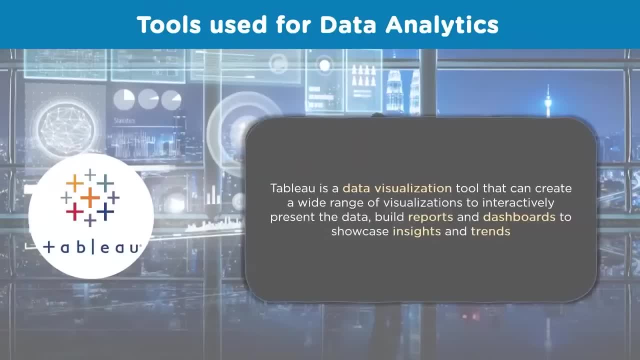 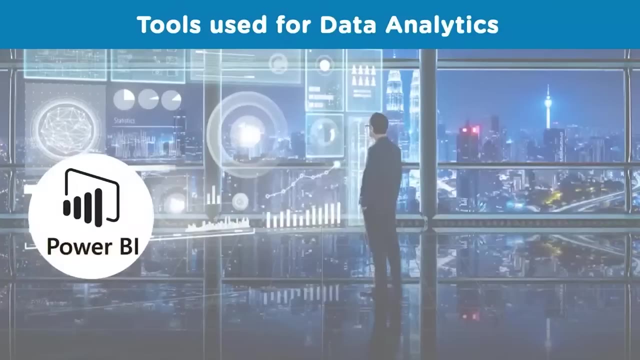 popular data visualization and analytics tools that helps you create a range of visualizations to interactively present the data, build reports and dashboards to showcase insights and trends. It can connect with multiple data sources and give hidden business insights and patterns. Then we have a. 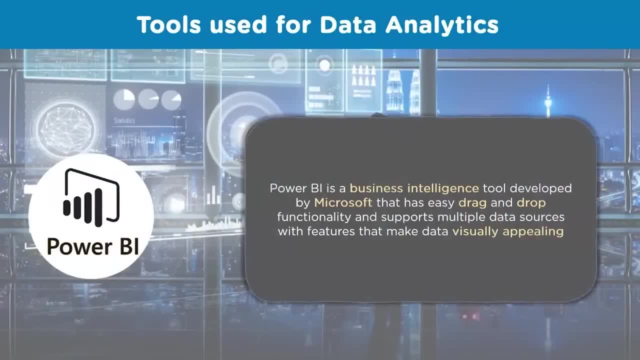 competitor of tableau, which is Power BI. Power BI is a business intelligence tool developed by Microsoft that has an easy drag-and-draw functionality and supports multiple data sources with features that make data visually appealing. Power BI supports features that help you ask questions to your data and get 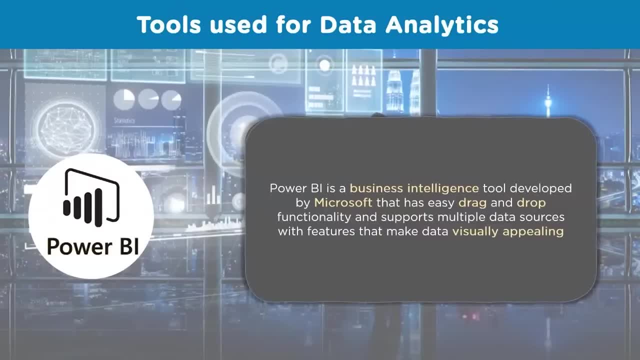 immediate insights. You can also forecast your data for predicting future trends. So the next tool is QlikView. QlikView provides interactive analytics with in-memory storage technology to analyze vast volumes of data and use data discoveries to support decision making. It provides social media discovery and 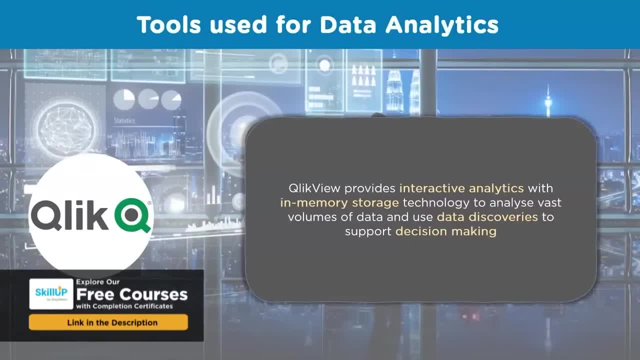 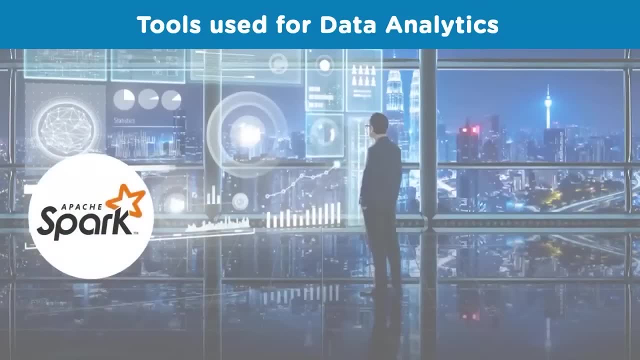 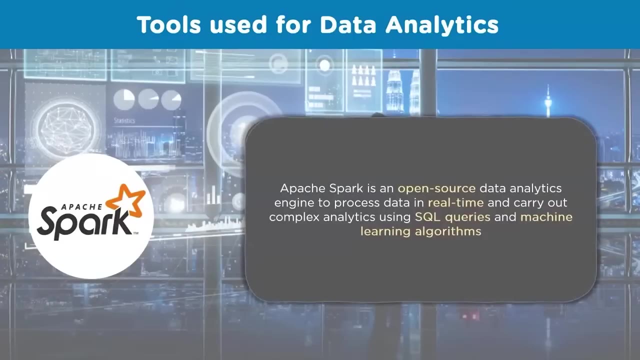 interactive guided analytics. It can manipulate huge datasets instantly with accuracy. Up next we have Apache spark. Apache spark is a highly popular data analytics tool that supports data analysis and analysis. Apache spark is an open source data analytics engine to process data in real time and carry out complex analytics using. 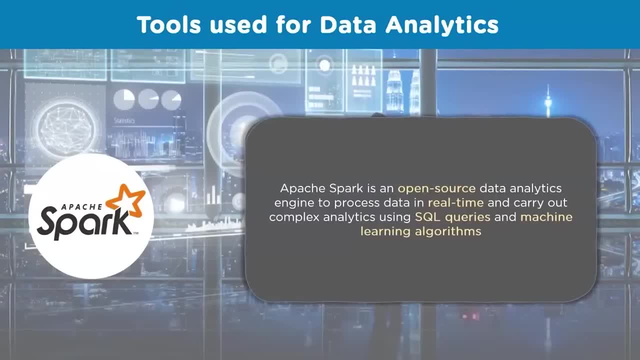 SQL queries and machine learning algorithms. It supports spark streaming for real time analytics and spark SQL for writing SQL queries. It also has spark ML lib, which is a library that has a repository of machine learning algorithms, and then it has graphics for graphical computation. And finally we 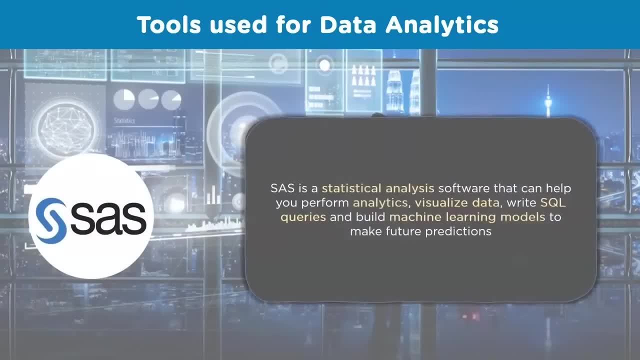 have SAS. SAS is a statistical analysis software that can help you perform analytics, visualize your data, write SQL queries, perform statistical analysis and build machine learning models to make future predictions. SAS empowers our customers to move the world forward by transforming data into intelligence. SAS- 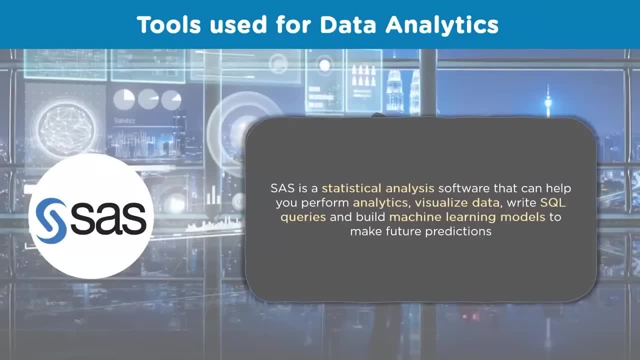 is investing a lot to drive software innovation for analytics. Gartner has positioned SAS as a magic quill for data analysis. SAS is a software innovation for analytics. Gartner has positioned SAS as a magic quadrant leader for data science and machine learning. Moving on to the 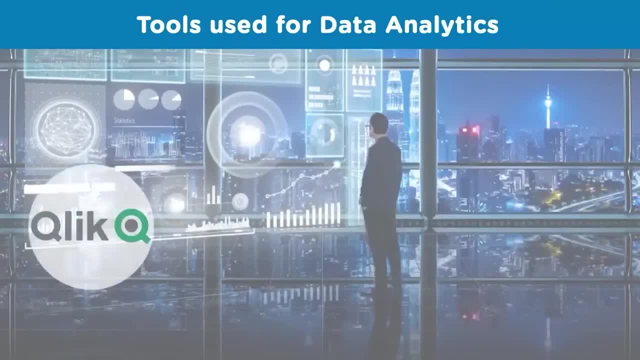 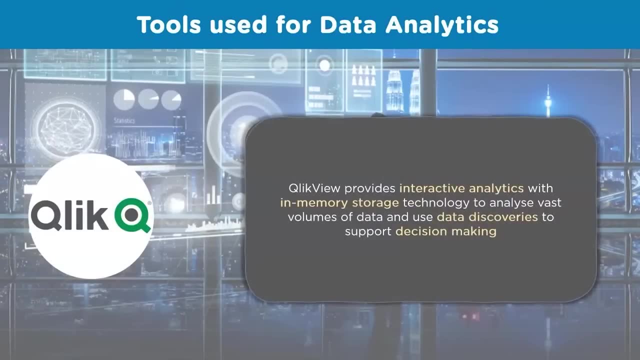 predicting future trends. so the next tool is click view. click view provides interactive analytics with in-memory storage technology to analyze vast volumes of data and use data discoveries to support decision making. it provides social media discovery and interactive guided analytics. it can manipulate huge data sets instantly with accuracy. 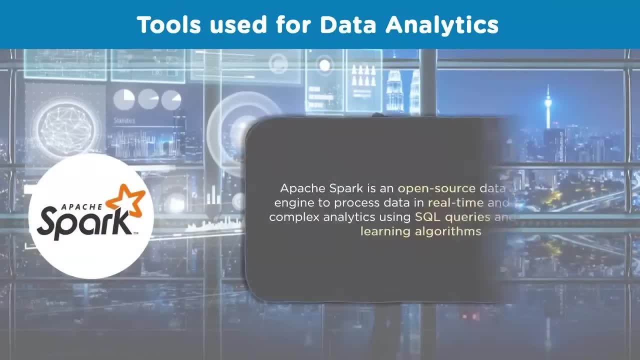 up. next we have Apache spark. Apache spark is an open-source data analytics engine to process data in real time and carry out complex analytics using sequel queries and machine learning algorithms. it supports spark streaming for real time analytics and spark SQL for writing SQL queries. it also has spark ML live. 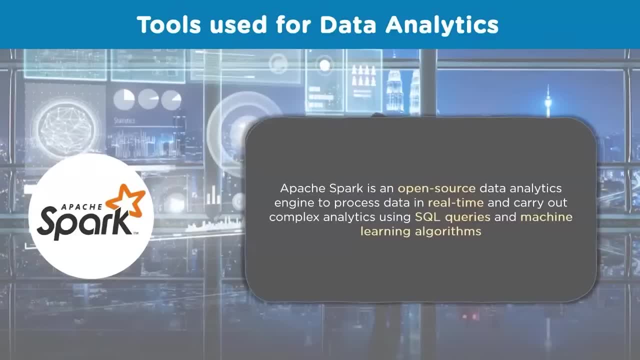 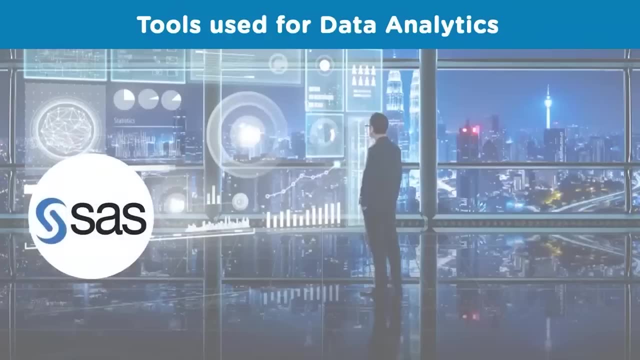 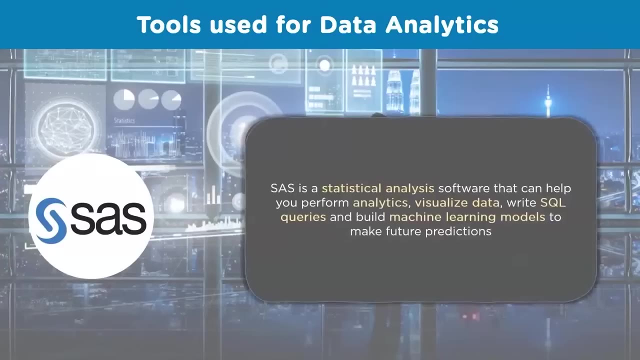 which is a library that has a repository of machine learning algorithms, and then it has graphics for graphical computation. and finally we have SAS. SAS is a statistical analysis software that can help you perform analytics, visualize your data, write SQL queries, perform statistical analysis and build machine learning models to make future predictions. SAS empowers our 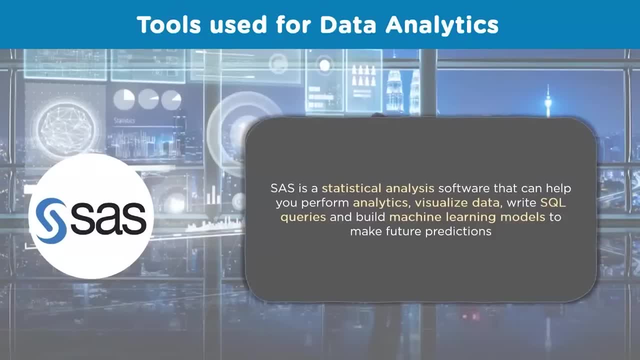 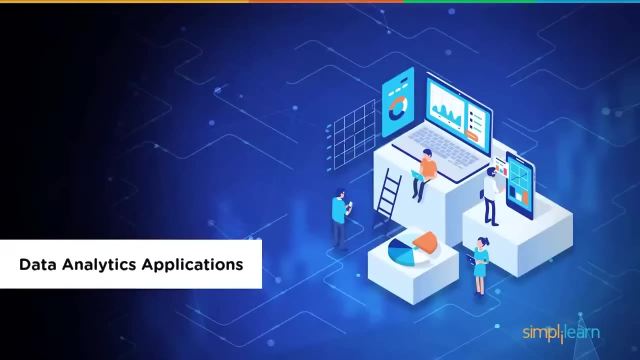 customers to move the world forward by transforming data into intelligence and transform data into intelligence. SAS is investing a lot to drive software innovation for analytics. Gartner has positioned SAS as a magic quadrant leader for data science and machine learning. moving on to the applications of data analytics, data analytics is being used in almost every sector of business. these 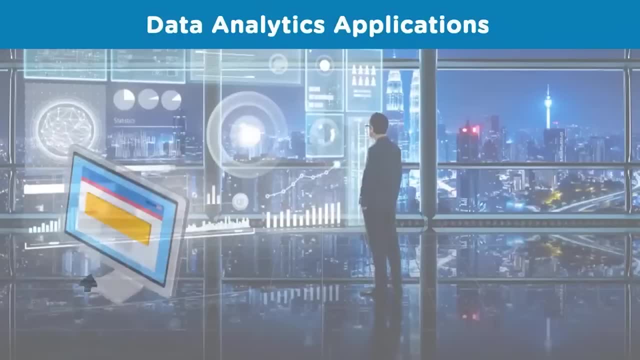 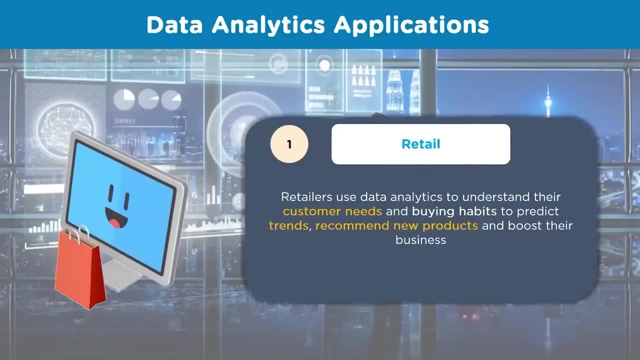 days. let's discuss a few of them. first, we have retail customers expect retailers to understand exactly what they need and when they need it. data analytics helps retailers meet those demands. retailers not only have an in-depth understanding of their customers, but they can also predict trends, recommend new products and boost profitability. retailers create 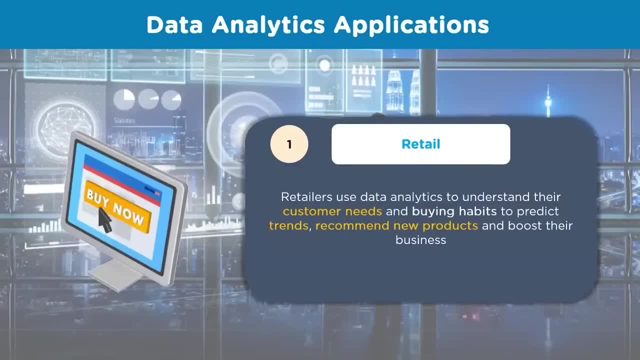 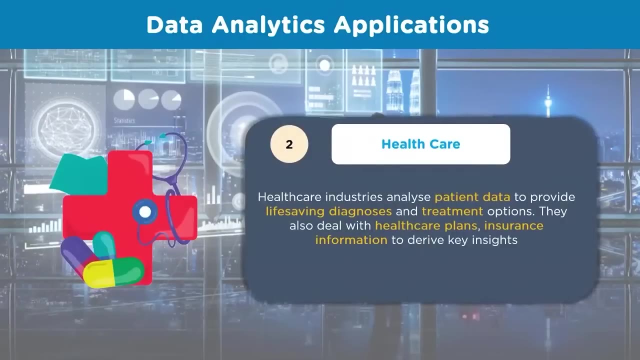 assortments based on customer preferences. invoke the most relevant engagement strategy for each customer. optimize supply chain and retail operations at every step of the customer journey. the second application is on health care. health care industries analyze patient data to provide life-saving diagnosis and treatment options. they also deal 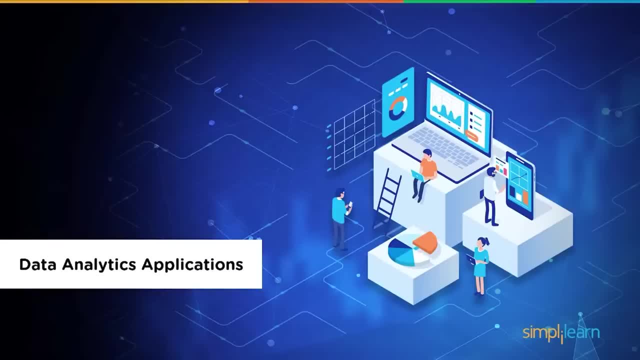 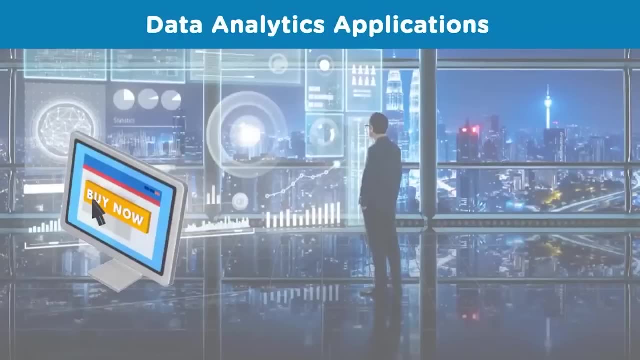 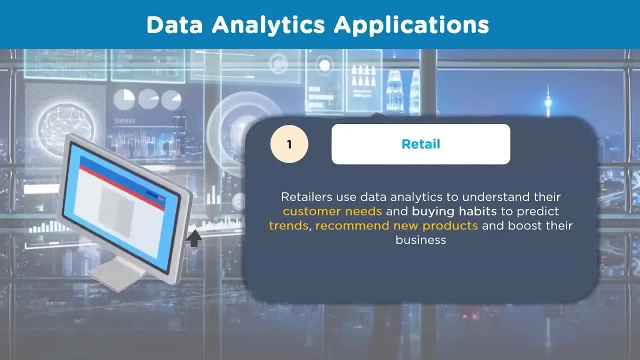 applications of data analytics. Data analytics is being used in almost every sector of business these days. Let's discuss a few of them. First, we have retail Customers expect retailers to understand exactly what they need and when they need it. Data analytics helps retailers meet those. 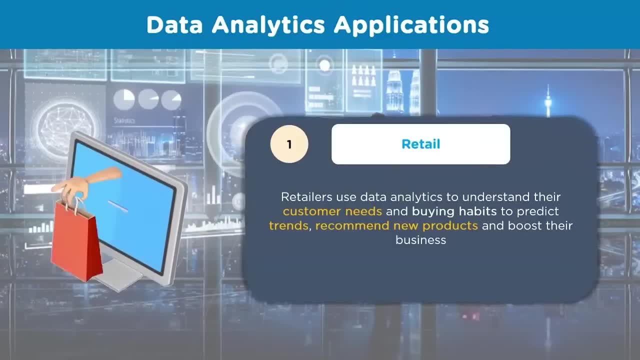 demands. Retailers not only have an in-depth understanding of their customers, but they can also predict trends, recommend new products and boost profitability. Retailers create assortments based on customer preferences, invoke the most relevant engagement strategy for each customer, optimize supply chain and. 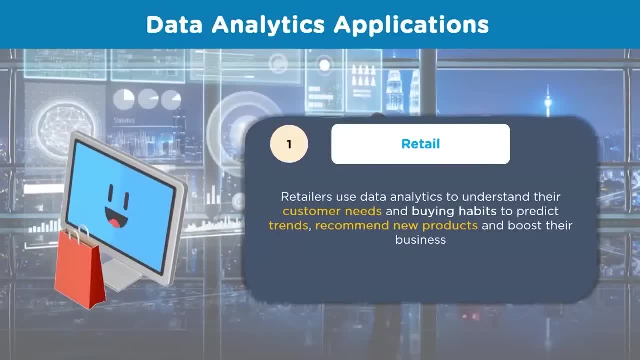 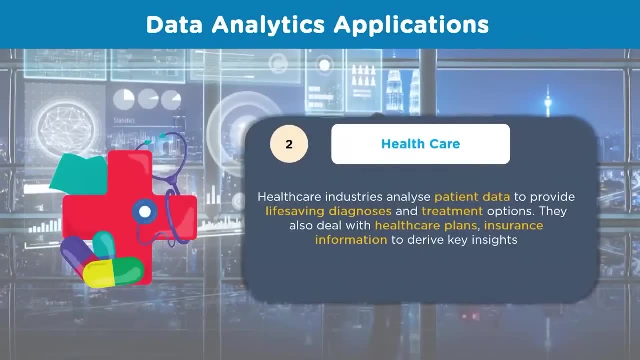 retail operations at every step of the customer journey. The second application is on healthcare. Healthcare industries analyze patient data, Ribbon and machine learning. For example, they are able to minimize the cost of packaging according to their consumption. They use artificial intelligence to provide life saving diagnoses and treatment options. They also deal with healthcare plans and insurance information to drive key insights. Using analytics, they can discover new drugs and come up with new drug development methods. Advanced analytics allows healthcare companies to improve patient outcomes and experience. Cancer cells and diabetic retinopathy can be discovered using medical imaging. 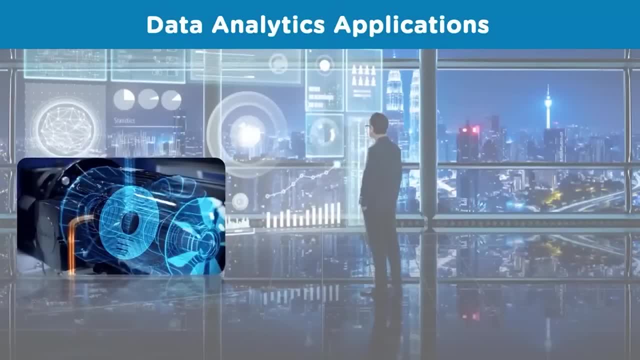 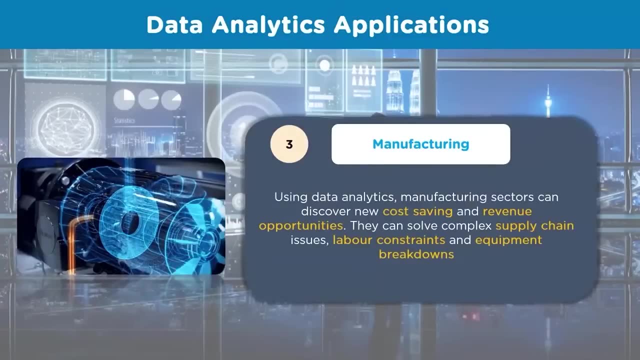 At number 3, we have manufacturing. For manufacturers, solving problem is nothing new. They fight with difficult problems and situations on a daily basis. From complex supply chains to motion applications, to labor constraints and equipment breakdowns. they deal with such problems on a regular basis. 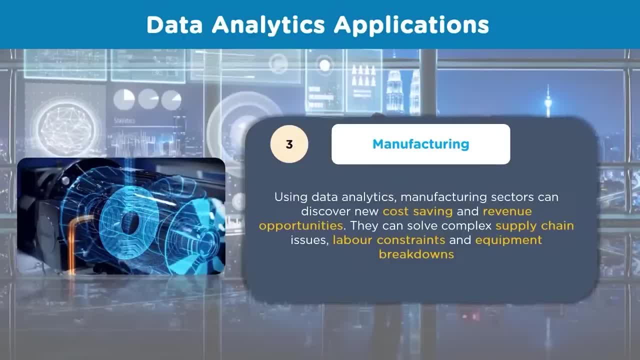 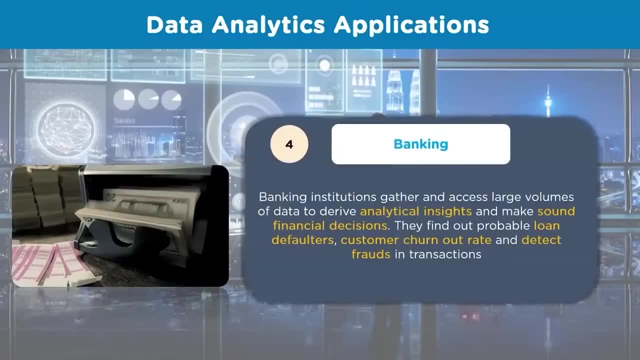 Using data analytics, manufacturing sectors can discover new cost-saving and revenue opportunities. The fourth application is related to the banking sector. Banking and financial institutions collect vast volumes of structured and unstructured data to derive analytical insights and make sound financial decisions. Using analytics, they can find out probable loan defaulters, customer churnout rate and 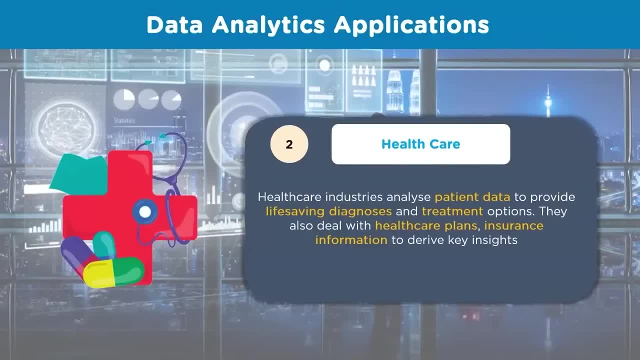 with health care plans and insurance information to drive key insights. using analytics, they can discover new drugs and come up with new drug development methods. advanced analytics allows health care companies to improve patient outcomes and experience. cancer cells and and diabetic retinopathy can be discovered using medical imaging. 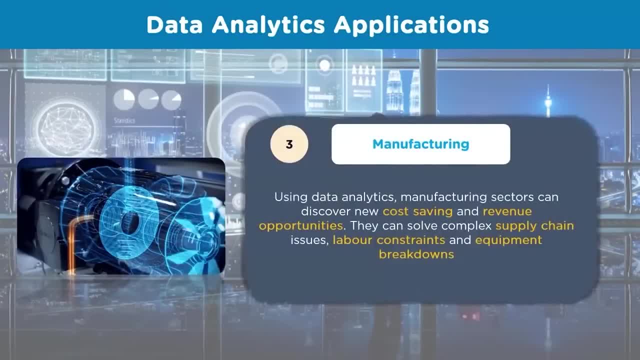 At number 3, we have manufacturing. For manufacturers, solving problem is nothing new. They fight with difficult problems and situations on a daily basis. From complex supply chains to motion applications, to labor constraints and equipment breakdowns. they deal with such problems on a regular basis. 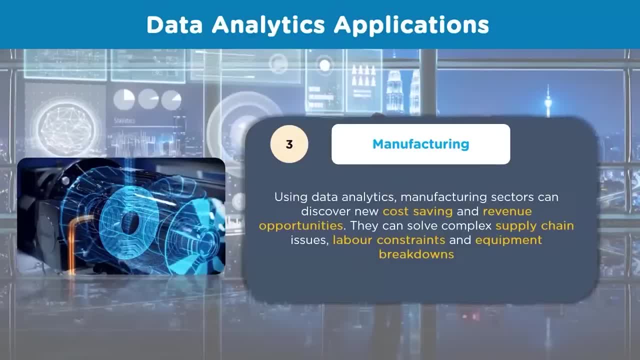 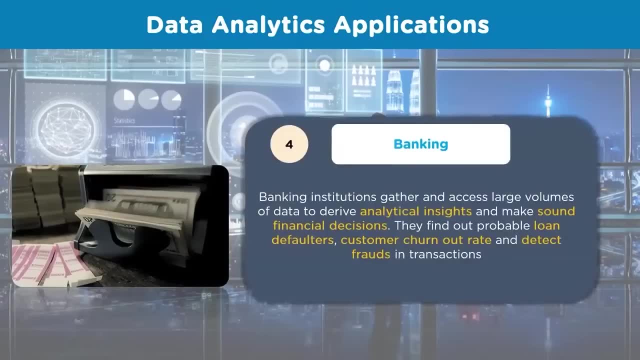 Using data analytics, manufacturing sectors can discover new cost-saving and revenue opportunities. The fourth application is related to the banking sector. Banking and financial institutions collect vast volumes of structured and unstructured data to derive analytical insights and make sound financial decisions. Using analytics, they can find out probable loan defaulters. customer churn-out rate. 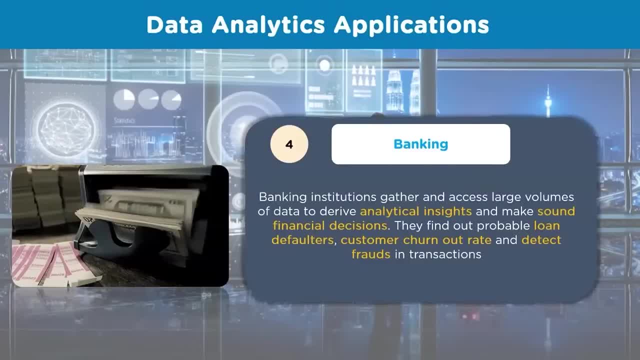 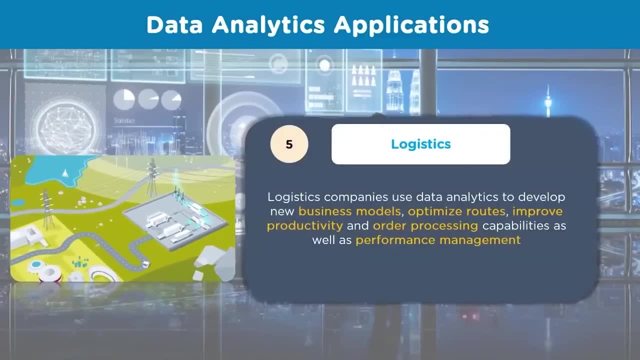 and detect fraudulent transactions immediately. The final application is based on logistics. Logistics companies use data analytics to develop new business models that can ease their business and improve productivity. They can optimize routes to ensure delivery reaches on time in a cost-efficient manner. They also focus on improving order processing capabilities, as well as performance management. 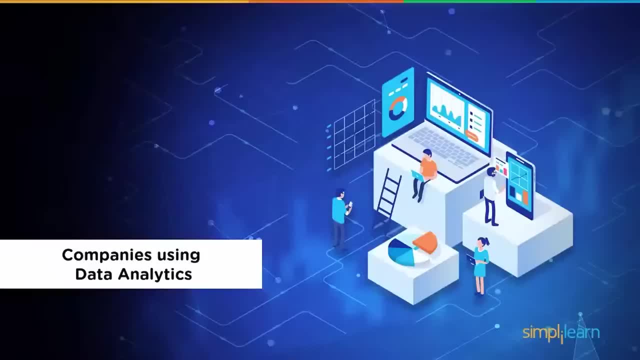 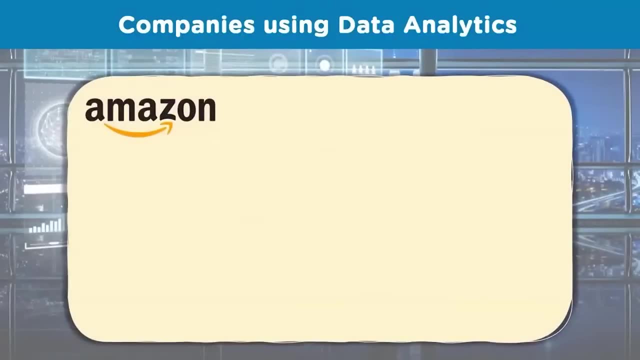 With that, now let's look at the companies using data analytics: 1. Amazon, 2. Accenture. 3. Cigna, 4. Cigna, 5. Cigna, 6. Cigna, 7. Cigna. 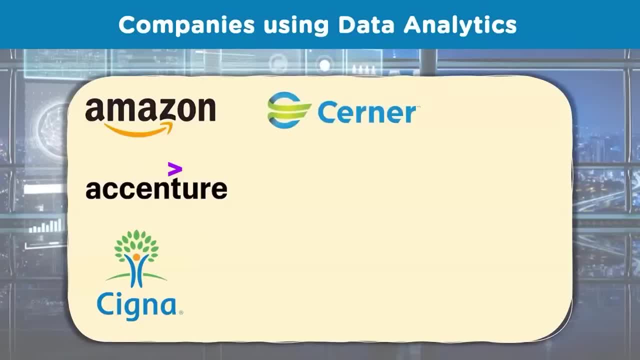 8. Cigna 9. Cigna 10. Cigna 11. Cigna 12. Cigna 13. Cigna 14. Cigna 15. Cigna 16.. 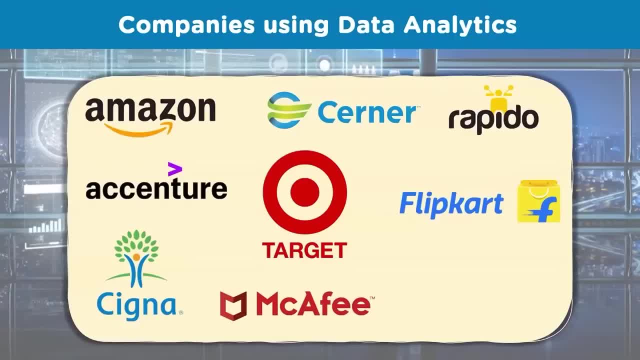 Cigna 17. Cigna 18.. Cigna 19.. Cigna 20.. Cigna 21.. Cigna 22.. Cigna 23.. Cigna 24. Cigna 25.. 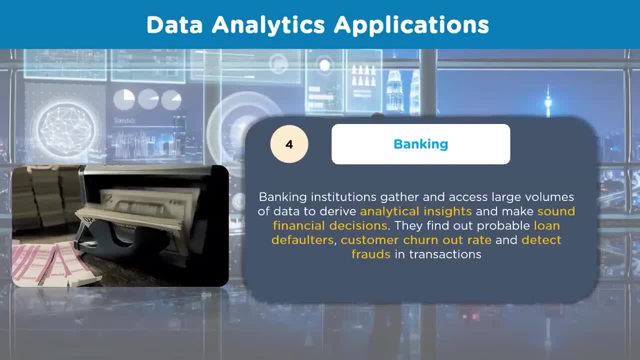 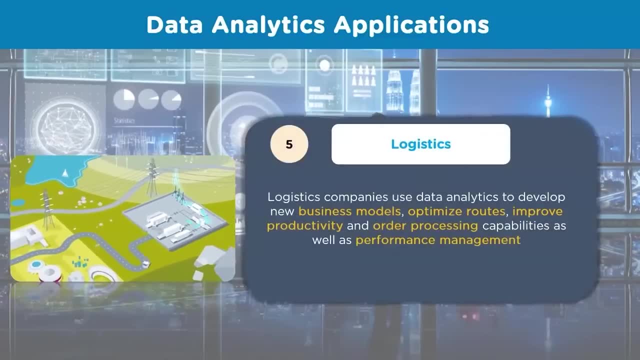 detect fraudulent transactions immediately. The final application is based on logistics. Logistics companies use data analytics to develop new business models that can ease their business and improve productivity. They can optimize routes to ensure delivery reaches on time in a cost-efficient manner. They also focus on improving order processing capabilities, as well as performance management. 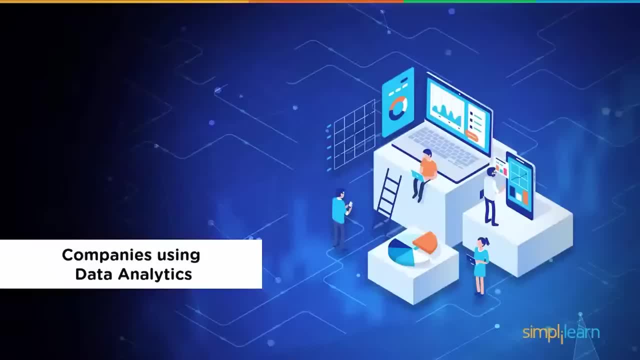 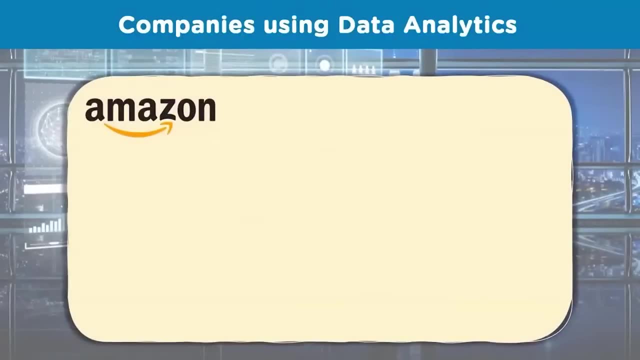 With that, now let's look at the companies using data analytics on a daily basis. So we have the e-commerce giant Amazon. We have the e-commerce giant Amazon. We have the e-commerce giant Amazon, Then we have Accenture, Then we have Accenture. 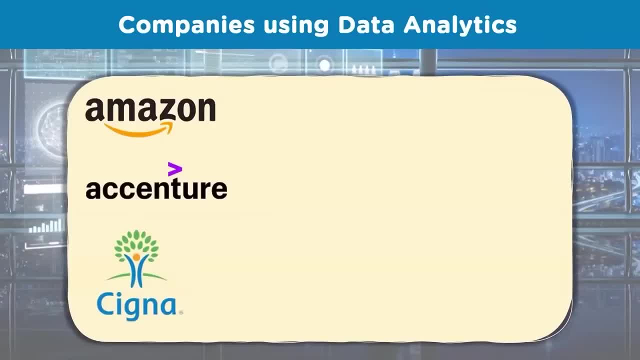 Followed by the American health care service organization, Cigna. Then we have the American supplier of health information technology solutions, services, devices and hardware, Cerner, Followed by Target and antivirus company McCafe. Next we have Rapido, which is an Indian bike rental company based in Bangalore. 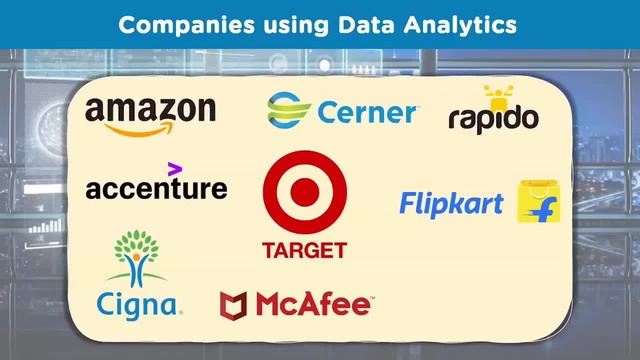 Next we have Rapido, which is an Indian bike rental company based in Bangalore. After that we have Flipkart, And the world's largest retail sales organization is Amazon. Next we have Amazon company Walmart. so sky's the limit on what you use it for. let's take a look at. 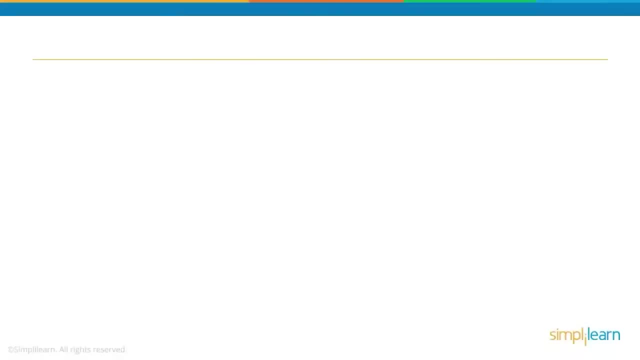 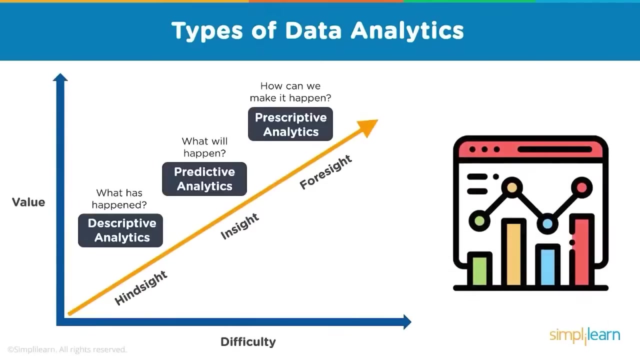 types of data analytics, and this can be broken up in so many ways, but we're going to start with looking at the most basic questions that you're going to be asking in data analytics, and the first one is: you want descriptive analytics. what has happened hindsight? how many cells per call ratio coming out of the? 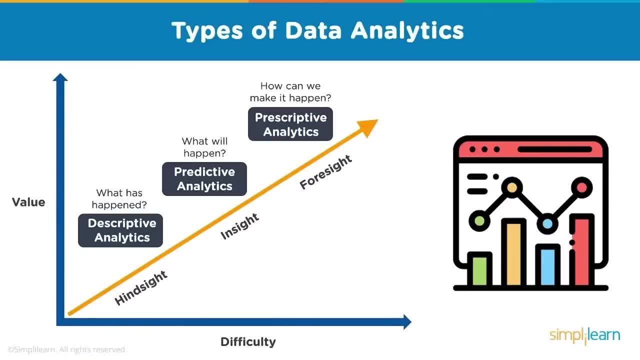 call center. if we have 500 tourists in a forest and you have a certain temperature, how many fires were started? how many times did the police have to show up to certain houses? all that's descriptive. the next one is predictive. predictive analytics is what will happen next. we want to predict. this is great if. 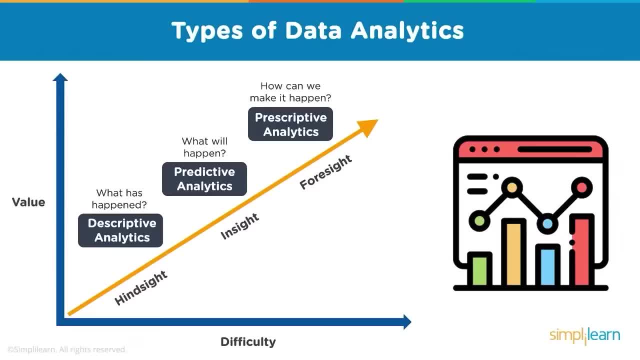 you have a ice cream store and you want to predict how many people to work at the ice cream store in a certain day based on the temperature coming up in the time of the year, and then one of the biggest growing and most important parts of the industry is now. 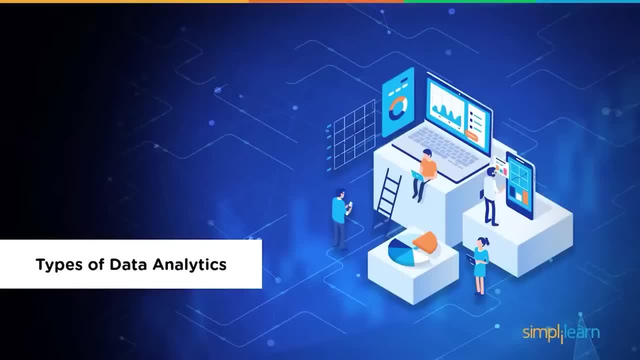 Cigna 26.. Cigna 26.. Cigna 27.. Cigna 28.. Cigna 29.. Cigna 30.. Cigna 31.. Cigna 32.. Cigna 33.. 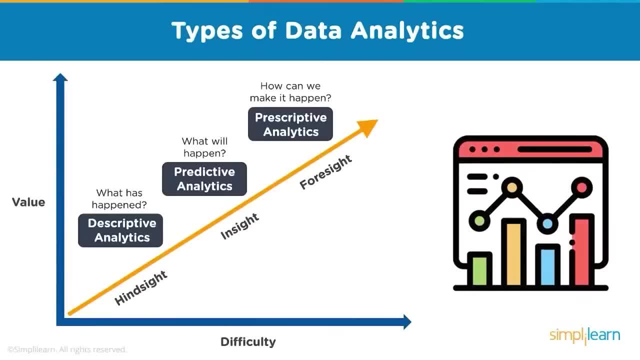 Cigna 34.. Cigna 35.. Cigna 36.. Cigna 37.. Cigna 38.. Cigna 39.. Cigna 40.. Cigna 41.. Cigna 42.. Cigna 43.. Cigna 45.. Cigna 46.. Cigna 47. Cigna 48.. Cigna 49.. Cigna 50.. Cigna 51.. Cigna 52.. 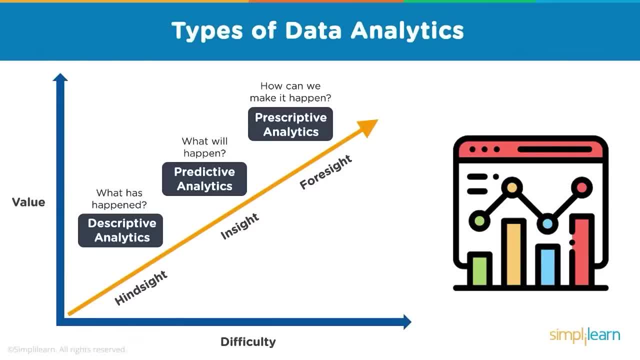 Cigna 53.. Cigna 54.. Cigna 55.. Cigna 56. Cigna 57.. Cigna 58.. Cigna 59. Cigna 60.. Cigna 61.. Cigna 62.. Cigna 63.. Cigna 64.. Cigna 65.. Cigna 67.. Cigna 68.. Cigna 69.. Cigna 70.. Cigna 71.. Cigna 72.. Cigna 73.. Cigna 74.. Cigna 75.. Cigna 76.. Cigna 78.. Cigna 79.. Cigna 80.. Cigna 91.. 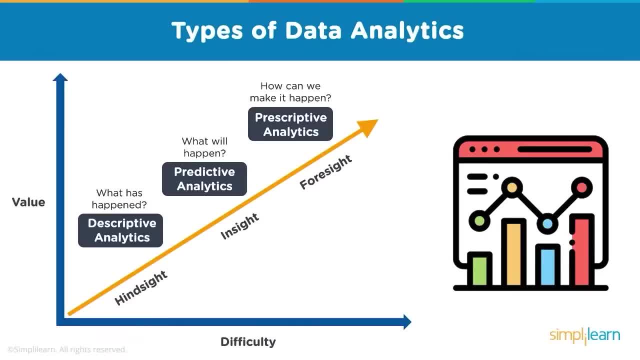 Cigna 92.. Cigna 93.. Cigna 94.. Cigna 95.. Cigna 96.. Cigna 97.. Cigna 98.. Cigna 99.. Cigna 100.. 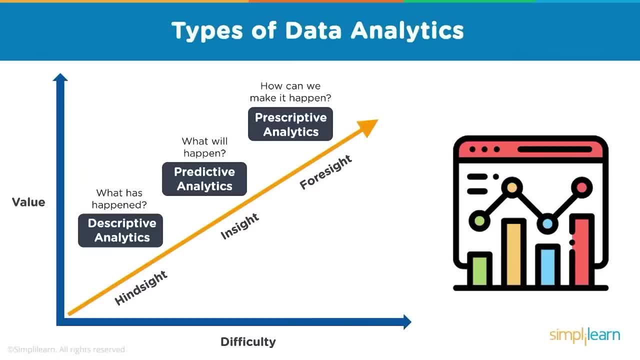 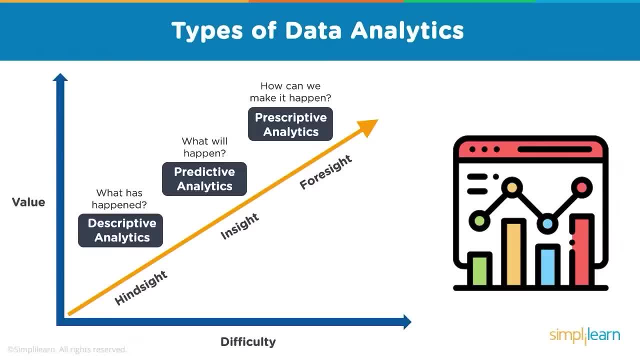 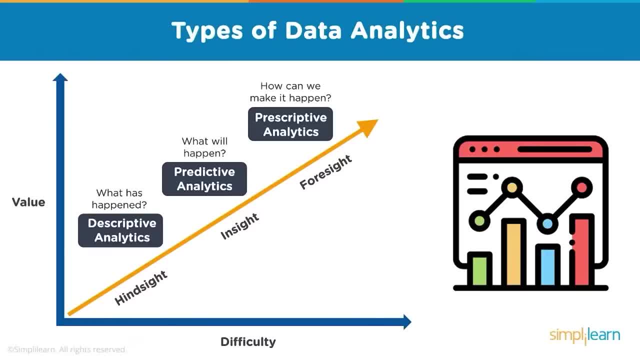 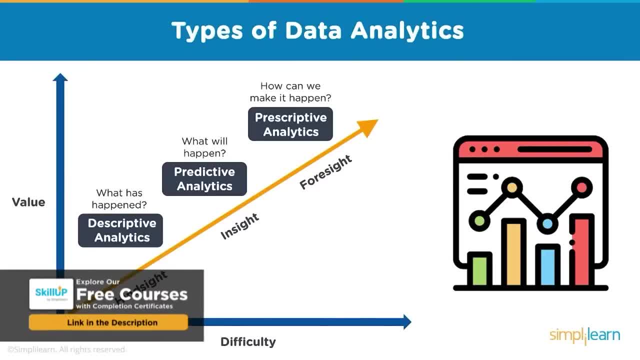 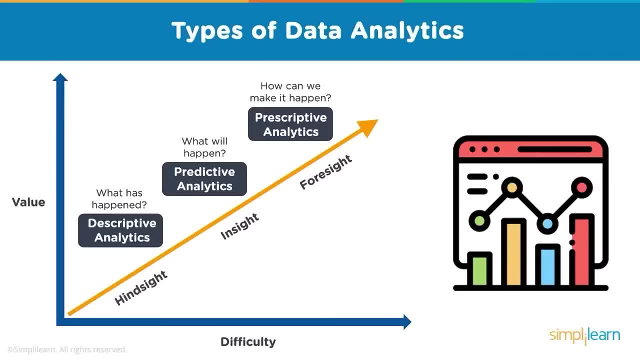 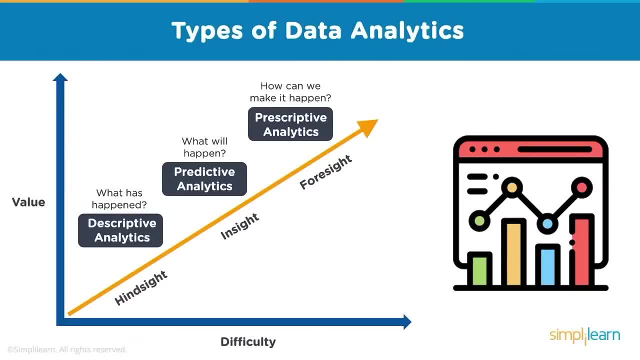 Cigna 100.. If it's not a car industry, what other industries are in that area? All those things are prescriptive. We're guessing. We're guessing. what can we do to fix it? What can we do to fix crime in an area with education? 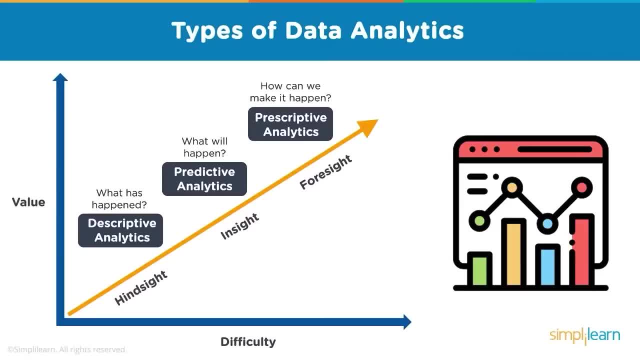 prescriptive analytics and you can think of that as combining the first two. we have descriptive and we have pre-dictive. then you get pre-scriptive analytics. how can we make it happen foresight? what can we change to make this work better in all the industries we looked at before we can start asking? 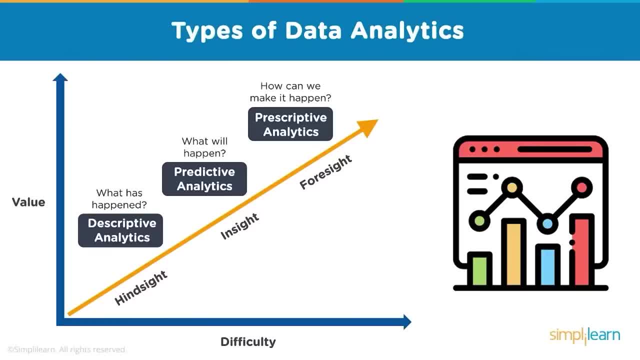 questions, especially in city development, there's a good one: if we want to have our city generate more income and we want that income to be commercial based, what kind of commercial buildings do we need to build in that area that are going to bring people over? do we need huge warehouse? 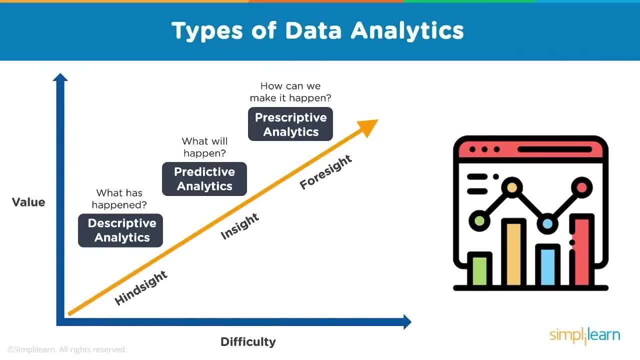 sales, Costco sales buildings, or do we need little mom-and-pop joints that are going to bring in people from the country to come shop there? or do you want an industrial setup? what do you need to bring that industry in there? is our car industry available in that area? if it's not a car industry, what other? 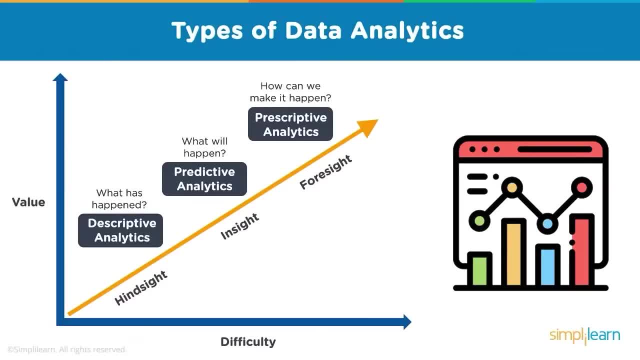 industries are in that area. all those things are prescriptive. we're guessing. we're guessing. what can we do to fix it? what can we do to fix crime? an area with education. what kind of education are we going to use to help people understand what's going on so that we lower the rate of crime and we help our 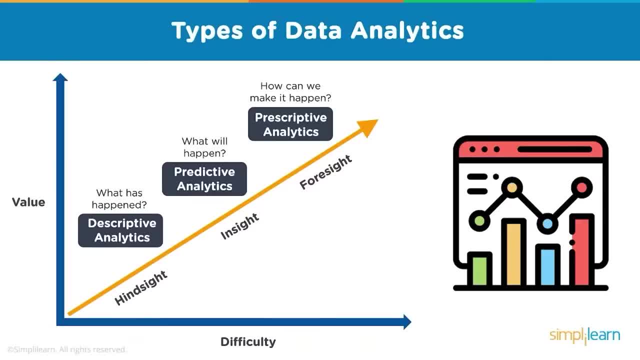 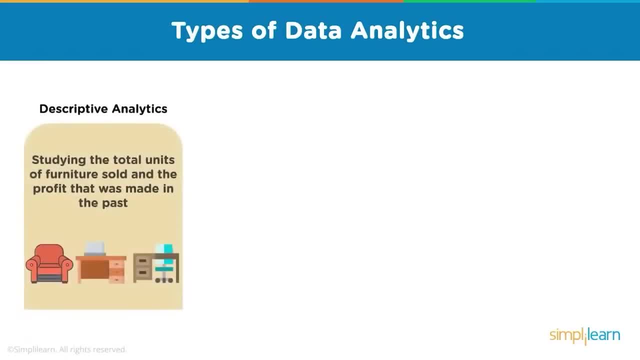 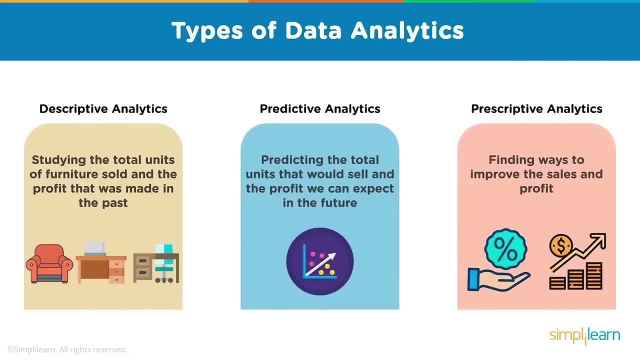 communities grow better. that's all prescriptive, it's all guessing. we want foresight into how can we make it happen, how can we make this better. and we really can't not go into enough detail on these three, because a lot of people stumble on this when they come in and are doing analytics. whether you're the 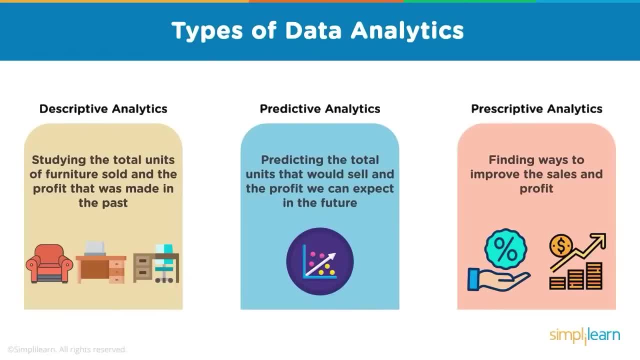 manager, shareholder or the data scientist coming in. you really need to understand the descriptive analytics, where you're studying the total units of furniture sold and the profit that was made in the past. here we go into predictive analytics, predicting the total units that would sell and the profit we can expect in the future. gear up for how many employees we need, how. 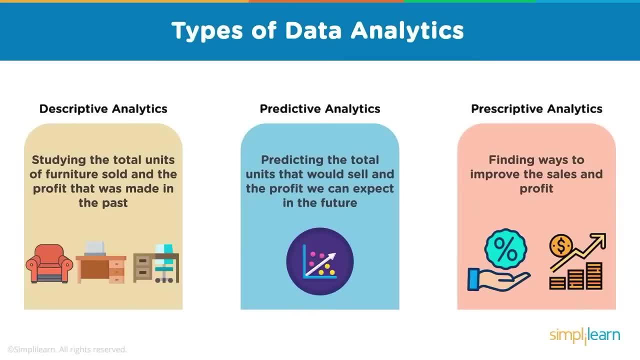 much money we're going to make and how much money we're going to make and prescriptive analytics finding ways to improve the sales and the profit so we can sell maybe a different kind of furniture. we're gonna guess at what the area is looking for and how that marketing is going to change. hello. 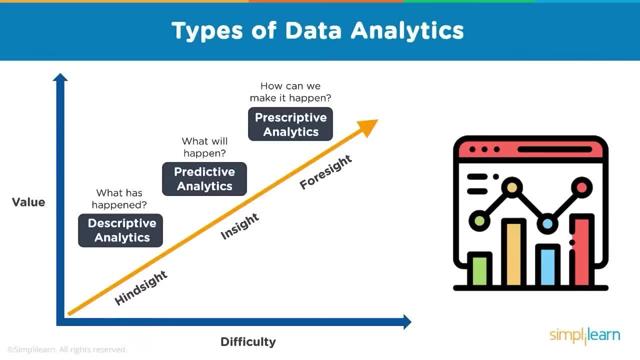 What kind of education are we going to use to help people understand what's going on, so that we lower the rate of crime and we help our communities grow better? That's all prescriptive, It's all guessing. We want foresight into how can we make it happen. 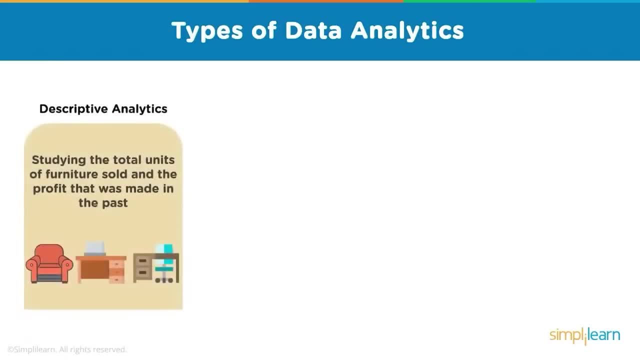 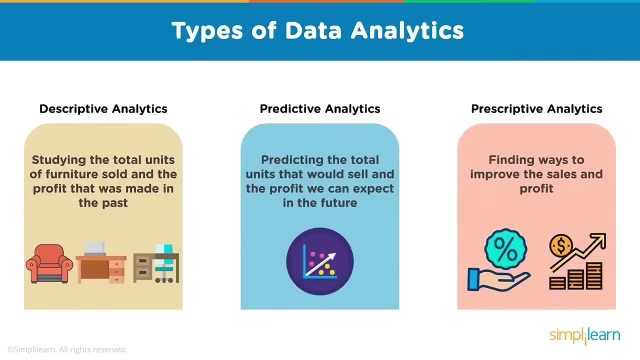 How can we make this better? And we really can't not go into enough detail on these three, because a lot of people stumble on this when they come in and are doing analytics, Whether you're the manager, shareholder or the data scientist coming in. 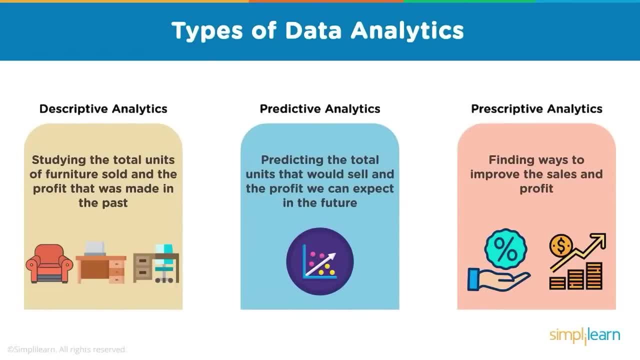 you really need to understand the descriptive analytics, where you're studying the total units of furniture sold and the profit that was made in the past. Here we go into predictive analytics, predicting the total units that would sell and the profit we can expect in the future. 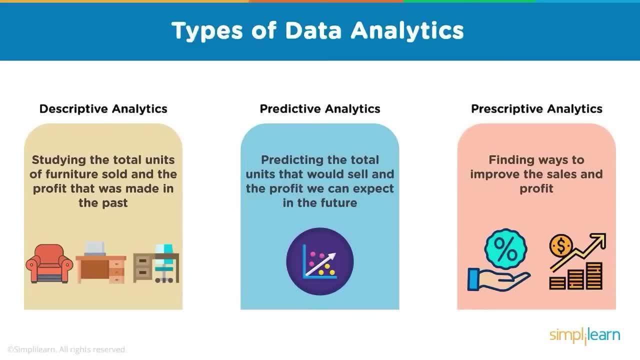 Gear up for how many employees we need, How much money we're going to make And prescriptive analytics finding ways to improve the sales and the profit so we can sell maybe a different kind of furniture. We're going to guess at what the area is looking for and how that marketing is going to change. 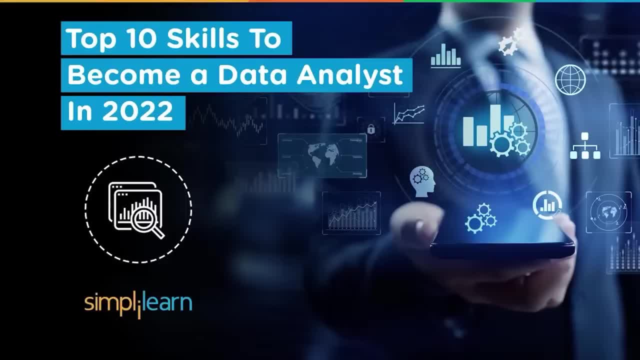 Hello everyone, We welcome you all to this video by Simply Learn. In today's session, we will learn a really interesting topic, that is, the top 10 skills to become a data analyst in 2022.. In today's digital world, data is being generated by computers. 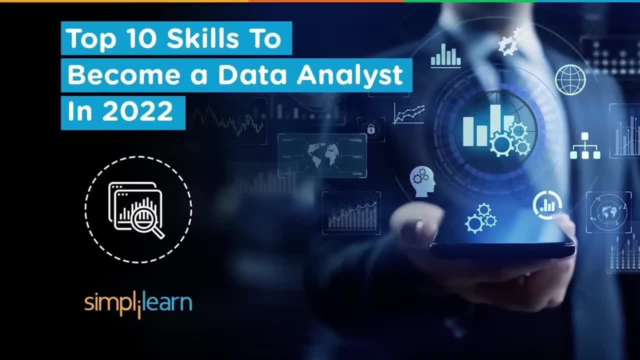 And companies and individuals every second, So the role of a data analyst holds supreme importance. So, if you're looking for a career in data analytics, this video will help you learn what a data analyst does and the various skills you need to possess to become a data analyst in 2022.. 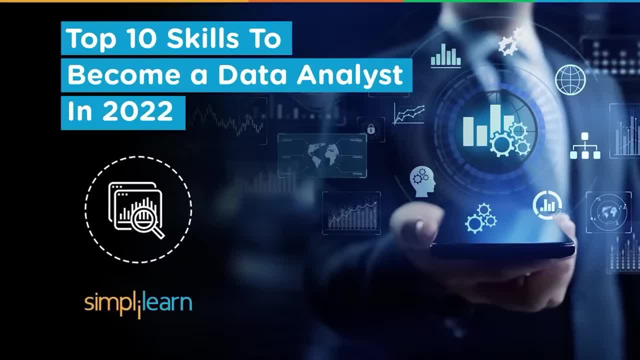 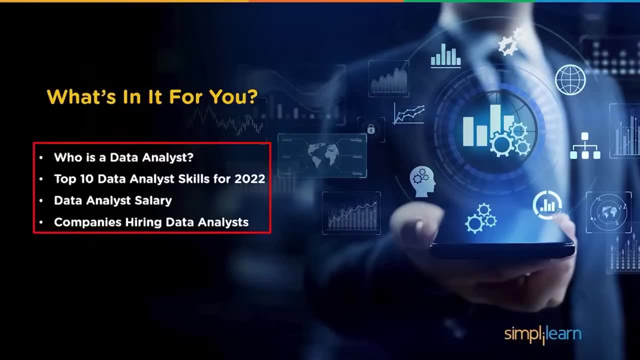 Before we get started, make sure you subscribe to the Simply Learn channel and hit the bell icon to never miss an update from us. Let's look at the agenda for this video. First, we will understand who a data analyst is. Then we will understand the top 10 data analyst skills for 2022. 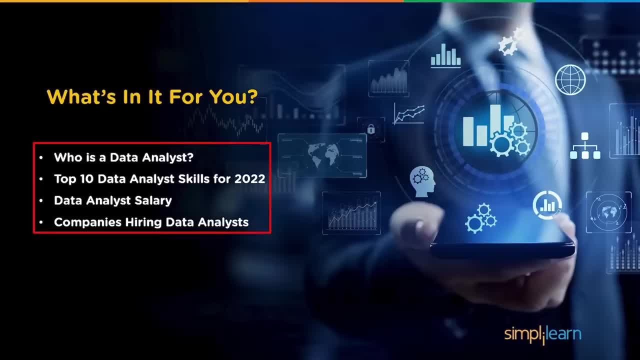 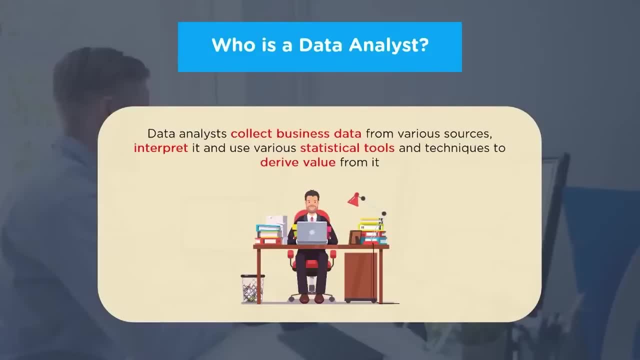 Moving on, we will look at the salary of a data analyst And, finally, we will look at the companies hiring data analysts. So now let's understand who is a data analyst. A data analyst is a professional who collects business data from various sources. 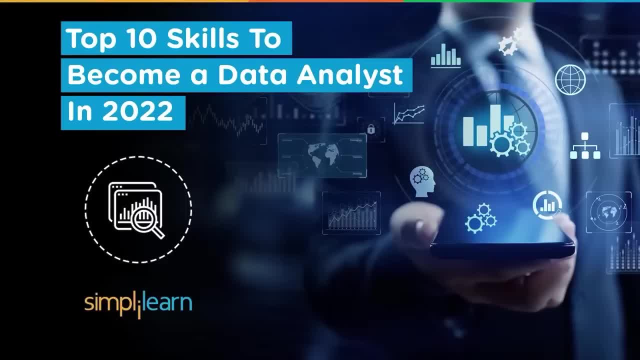 everyone. we welcome you all to this video by simply learn. in today's session, we will learn a really interesting topic, that is, the top 10 skills to become a data analyst in 2022. in today's digital world, data is being generated by companies and individuals. 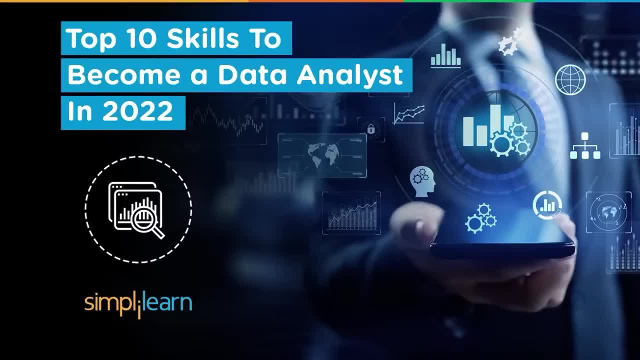 every second, so the role of a data analyst holds supreme importance. so if you're looking for a career in data analytics, this video will help you learn what a data analyst does and the various skills you need to possess to become a data analyst in 2022. before we get started, make sure you subscribe to the. 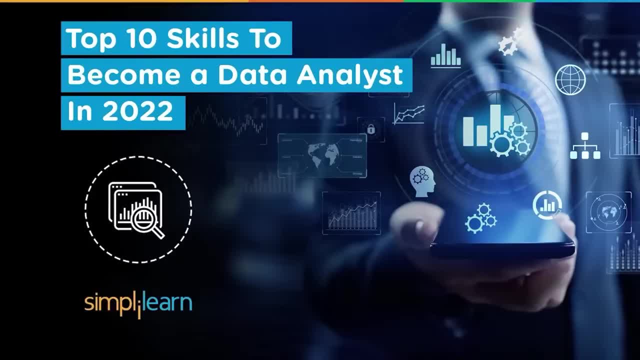 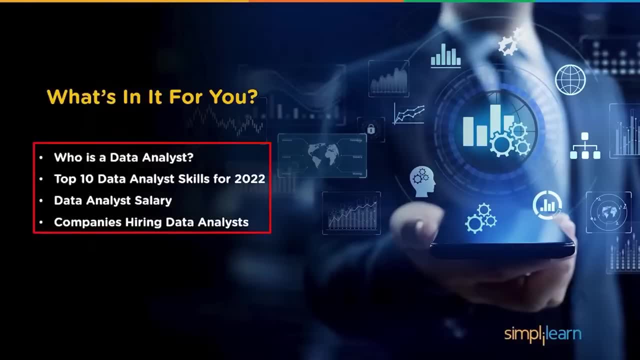 simply learn, channel and hit the bell icon to never miss an update from us. let's look at the agenda for this video. first, we will understand who a data and list is. then we will understand the top 10 data analyst skills for 2022. moving on, 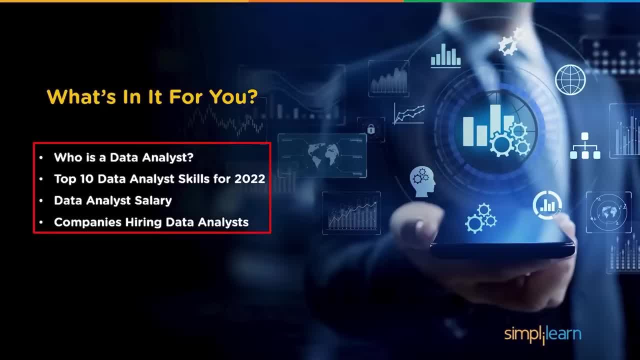 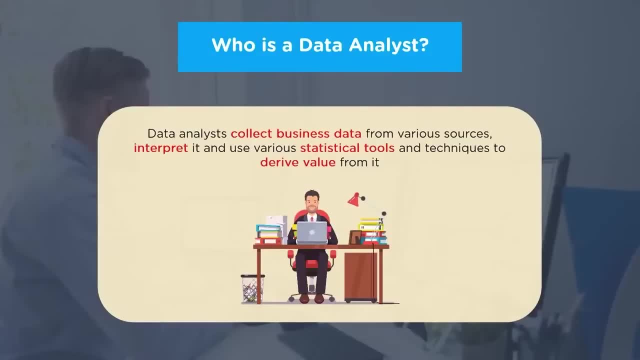 we will look at the salary of a data analyst and, finally, we will look at the companies hiring data analysts. so now let's understand who is the data analyst. a data analyst is a professional who collects business data from various sources, interprets it and uses various statistical tools and techniques to 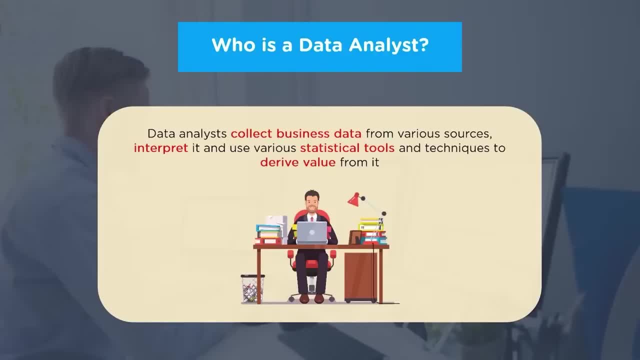 extract insights and useful information from it. they acquire data from primary or secondary data sources and maintain databases. they also recognize and understand the organization's goal and collaborate with different team members, such as programmers, business analysts and data scientists, to build an effective solution to a business problem. now, with this basic understanding of who, 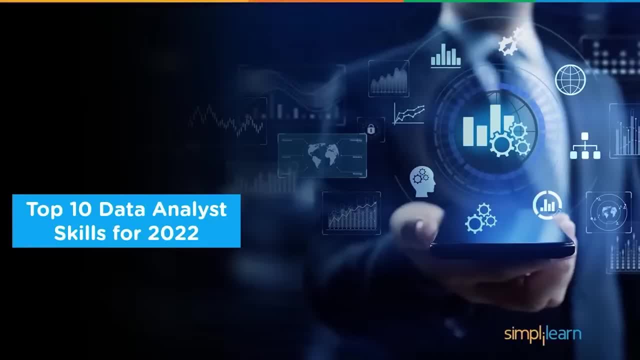 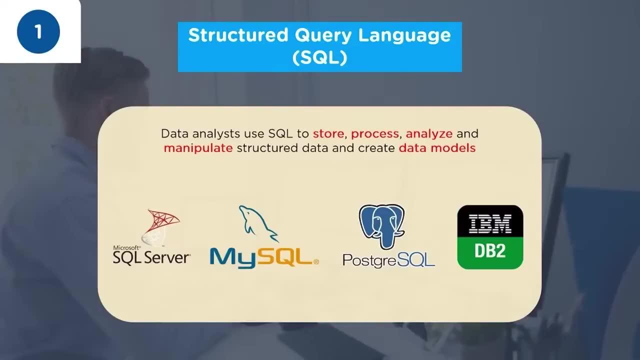 a data analyst is. let's learn the top 10 data analyst skills for 2022. at number one, we have structured query language, or SQL. SQL is a top skill that every data analyst should have. data analysts use SQL commands and functions to store, process, analyze and manipulate structured data. 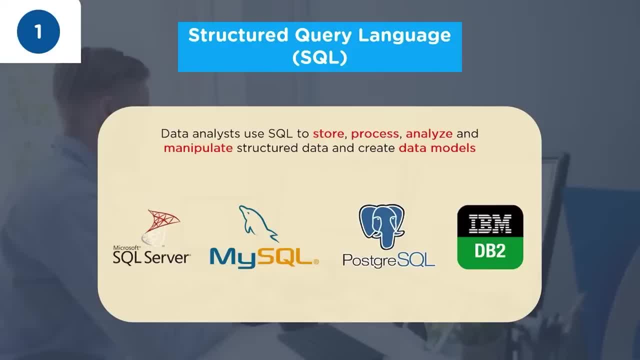 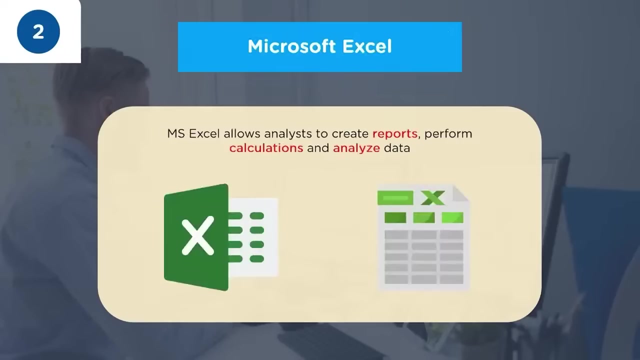 using relational and no sequel databases. they also build data models and write complex equal queries and scripts to gather and extract information from several databases and data warehouses. some of the popular databases a data analyst should be familiar with are Microsoft SQL server, MySQL, PostgreSQL and IBM DB to. the second important skill for a data analyst is Microsoft Excel. 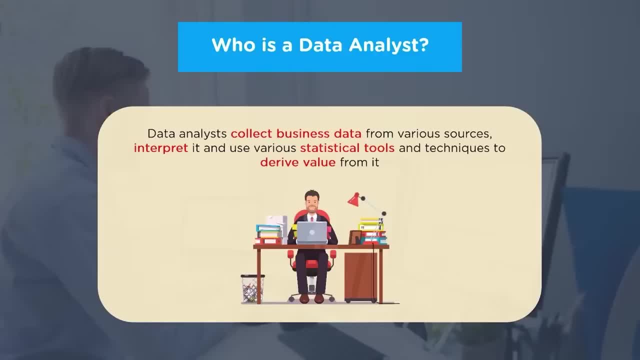 interprets it and uses various statistical tools and techniques to extract insights and useful information from it. They acquire data from primary or secondary data sources and maintain databases. They also recognize and understand the organization's goal and collaborate with different team members, such as programmers, business analysts and data scientists, to build an effective solution to a business problem. 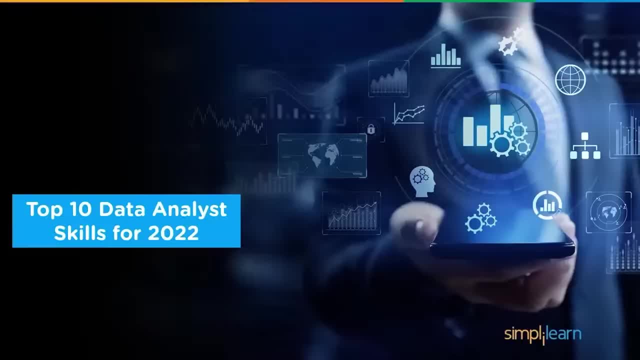 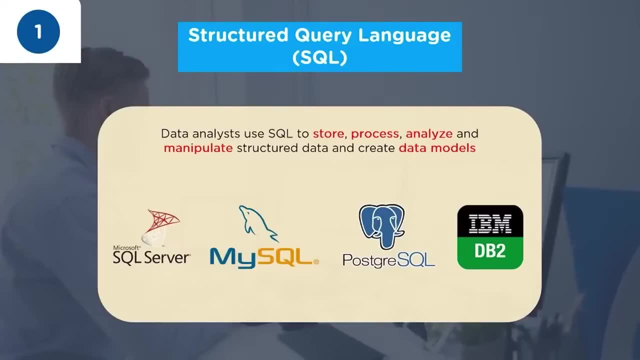 Now, with this basic understanding of who a data analyst is, let's learn the top 10 data analyst skills for 2022.. At number one, we have Structured Query Language, or SQL. SQL is a top skill that every data analyst should have. 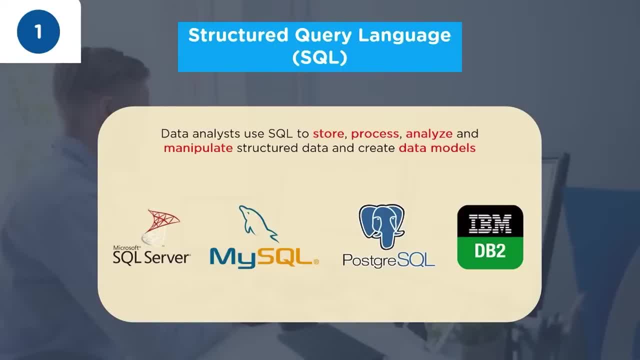 Data analysts use SQL commands and functions to store, process, analyze and manipulate structured data using relational and NoSQL databases. They also build data models and write complex SQL queries and scripts to gather and extract information from several databases and data warehouses. Some of the popular databases: 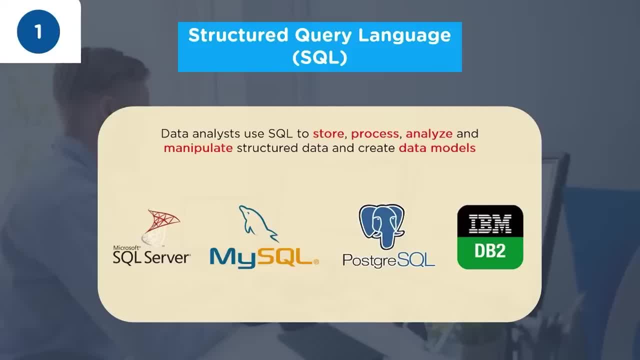 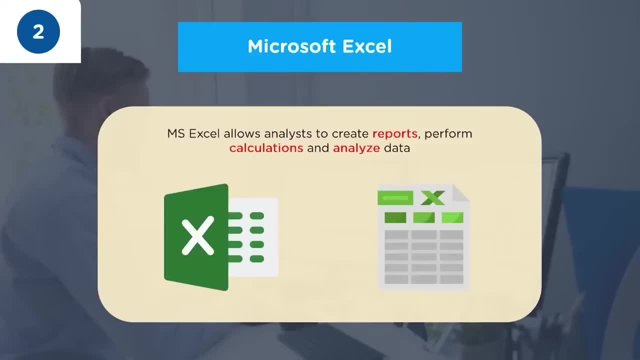 such as Google, Google, Google and Google are. the most popular databases a data analyst should be familiar with are Microsoft SQL Server, MySQL, PostgreSQL and IBM DB2.. The second important skill for a data analyst is Microsoft Excel. Microsoft Excel is one of the most popular and oldest spreadsheet applications for creating reports. 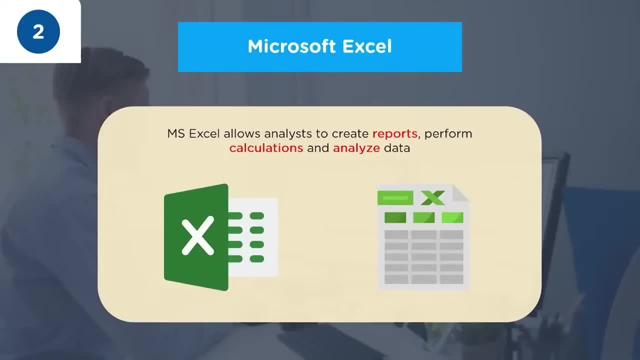 performing calculations and analyzing data. Data analysts need to know how to handle tabular data in Excel, so they should be aware of features like sorting, filtering, conditional formatting, pivot tables, what-if analysis and functions such as SUMIFs and COUNTIFS. 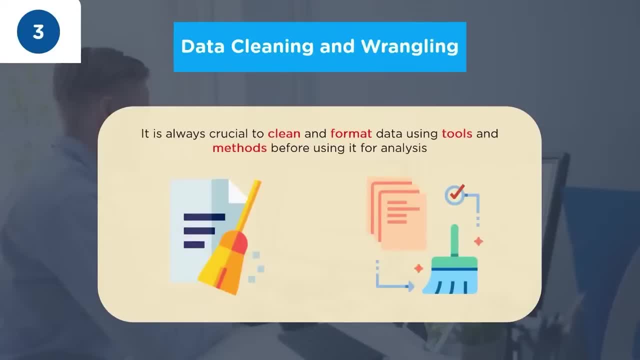 The third crucial data analyst skill for 2022 is data cleaning and wrangling. Usually, the data collected by analysts from various heterogeneous sources is often messy and contains a lot of missing values, So it is always crucial to clean the data and remove noise. 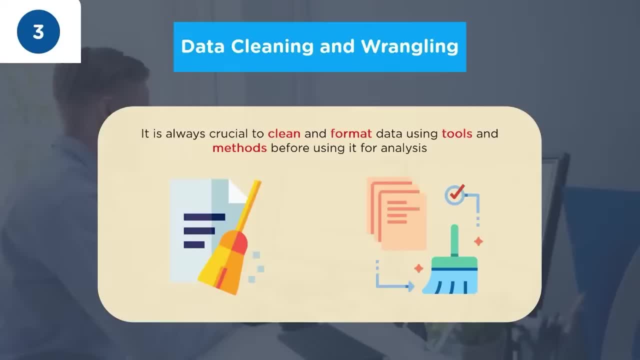 missing or erroneous elements. It is also important to know how to manage data, and it is important to format data using tools and methods before using it for analysis. They are responsible for data mining as well. The data mined from various sources are organized in order to obtain new information from it. 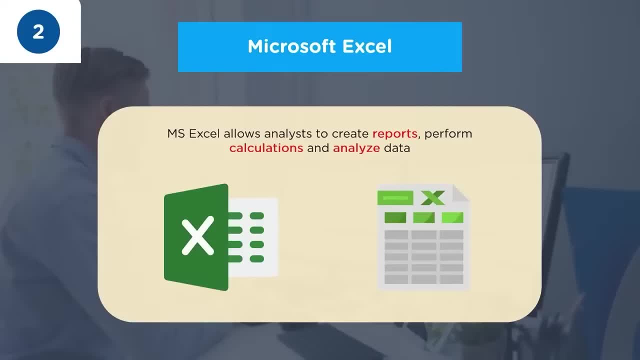 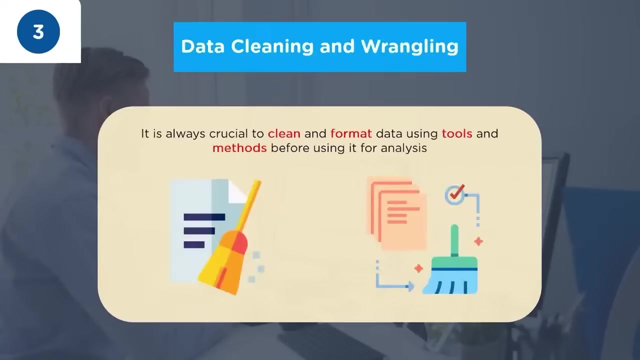 Microsoft Excel is one of the most popular and oldest spreadsheet applications for creating reports, performing calculations and analyzing data. data analysts need to know how to handle tabular data in Excel, so they should be aware of features like sorting, filtering, conditional formatting, pivot tables, what-if analysis and functions such as summifs and countifs. the third crucial. 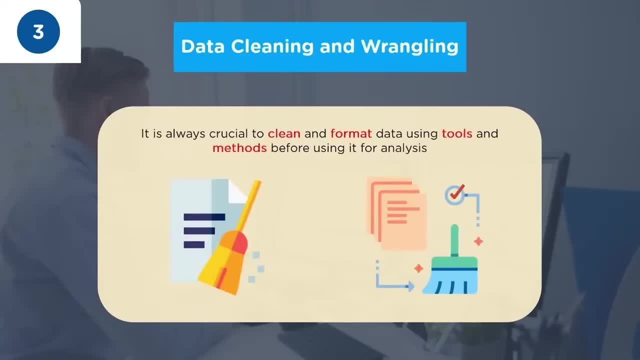 data analyst skill for 2022 is data cleaning and wrangling. usually, the data collected by analysts from various heterogeneous sources is often messy and contains a lot of missing values, so it is always crucial to clean the data and remove noise, missing or erroneous elements. it is also important to format. 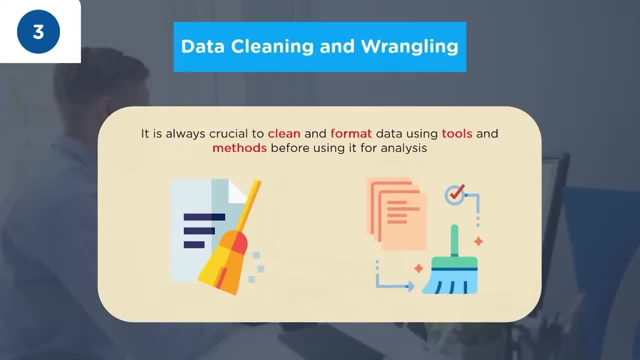 data using tools and methods before using data analysis to build a data analysis, before using it for analysis. they are responsible for data mining as well. the data mined from various sources are organized in order to obtain new information from it. some of the tools you need to know for data cleaning and. 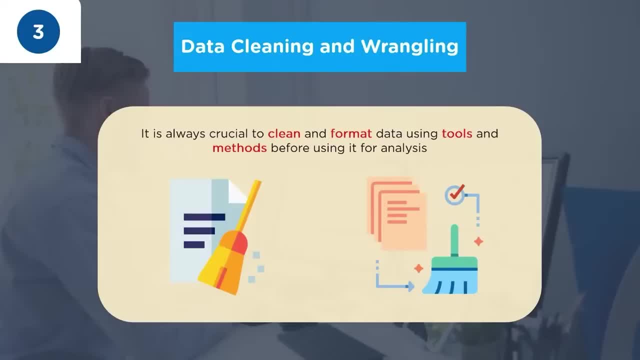 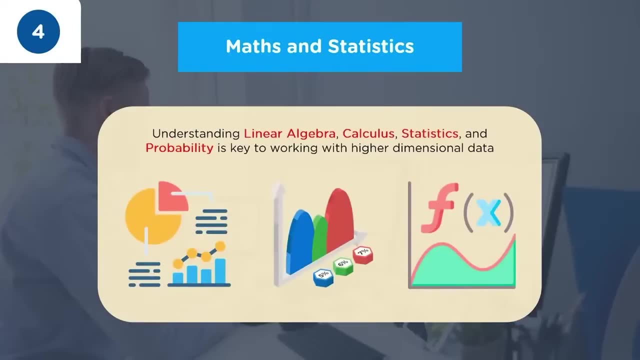 wrangling our Excel power query and open refine. the fourth skill on our list is mathematics and statistics. data analysts often work on data for higher dimensions that are greater than three. in order to interpret such data, they need to be good at linear algebra and calculus. they also build predictive models and 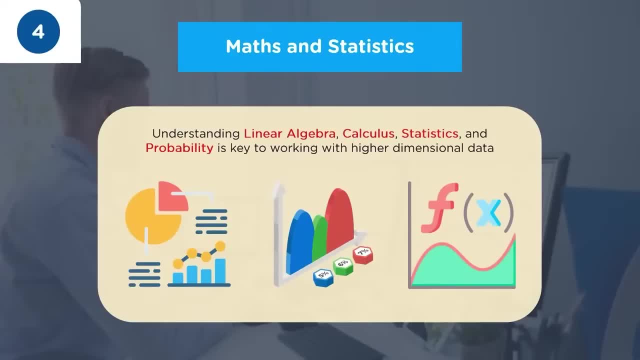 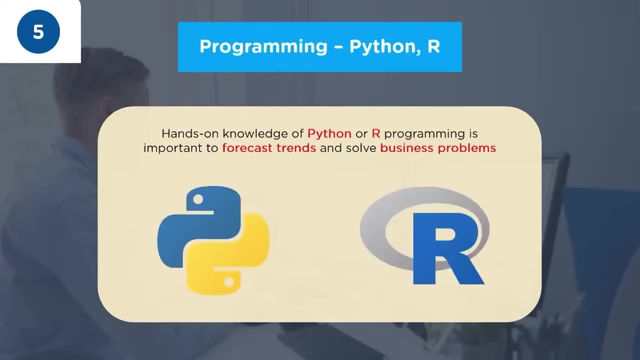 statistical models such as linear regression, logistic regression, knife base and k-means clustering. in order to understand the working of these algorithms, they must have knowledge about statistics and probability. coming to the fifth important skill for a data analyst in 2022, we have programming. data analysts need to master at least one programming language, preferably Python. 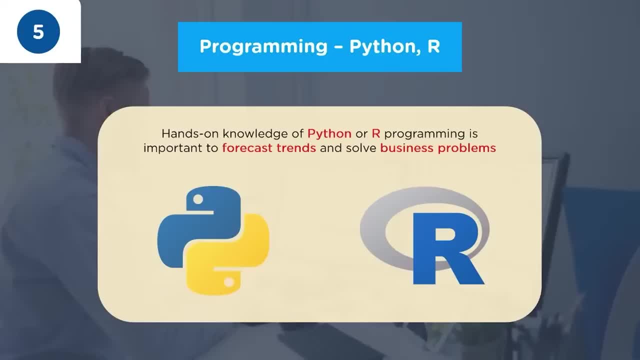 or R in order to work with complex business problems. analysts need to write scripts and user-defined functions to automate tedious tasks. Python and R language provide a collection of different libraries and packages, such as numpy, pandas, dplyr, matplotlib, ggplot, which data analysts can use to discover trends. 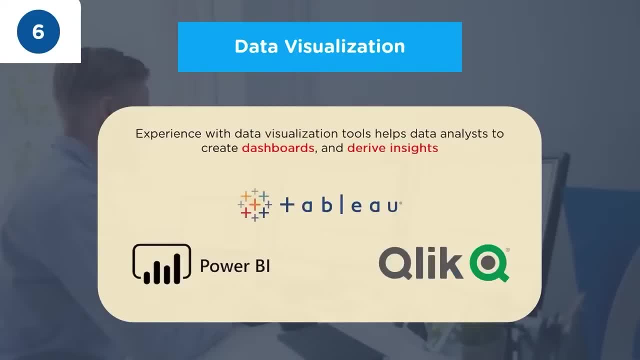 and patterns from complex data sets. after this we have data visualization as a sixth skill. another data analyst job role is to visualize large-scale data, volumes of data and prepare summary reports and dashboards for the leadership team and clients so that they can make timely business decisions to do. 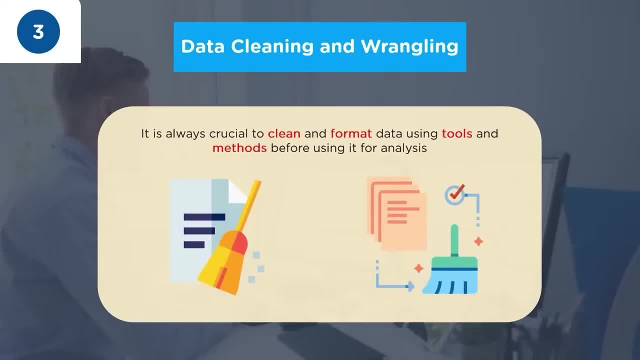 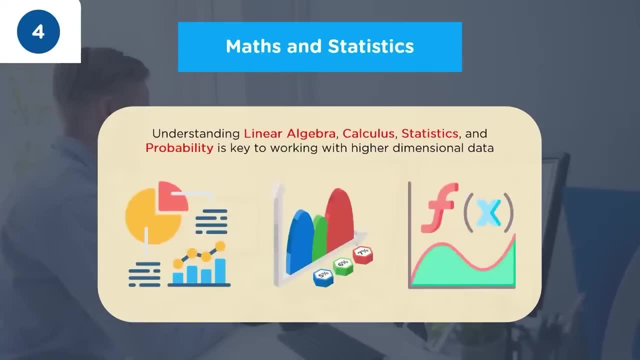 Some of the tools you need to know for data cleaning and wrangling are Excel, Power Query and OpenRefine. The fourth skill on our list is mathematics and statistics. Data analysts often work on data for higher dimensions that are greater than three, In order to interpret such data. 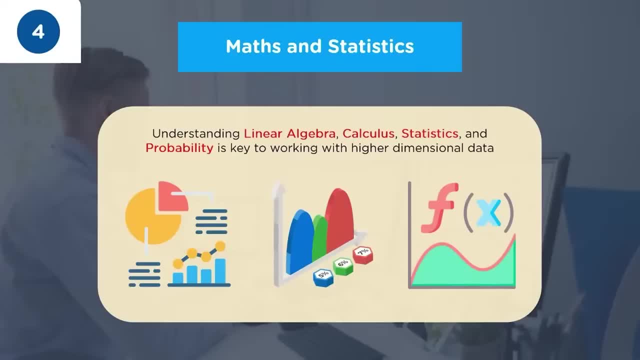 they need to be good at linear algebra and calculus. They also build predictive models and statistical models such as linear regression, logistic regression, knife base and k-means clustering. In order to understand the working of these algorithms, they must have knowledge about statistics and probability. 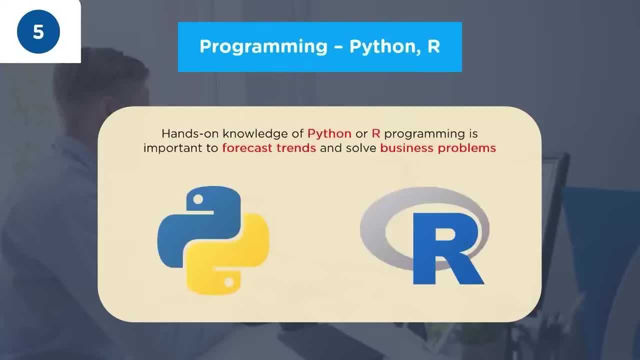 Coming to the fifth important skill for a data analyst in 2022, we have programming. Data analysts need to master at least one program or programming language, preferably Python or R, In order to work with complex business problems. analysts need to write scripts and user-defined functions to automate tedious tasks. 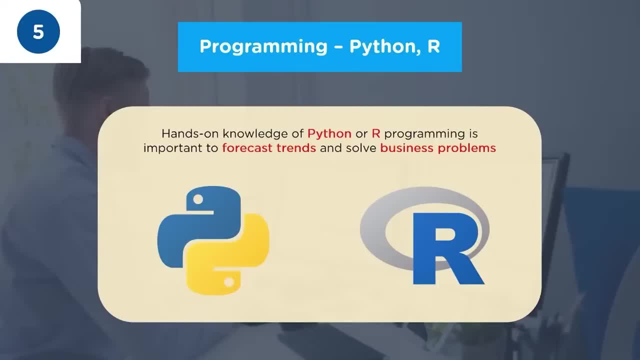 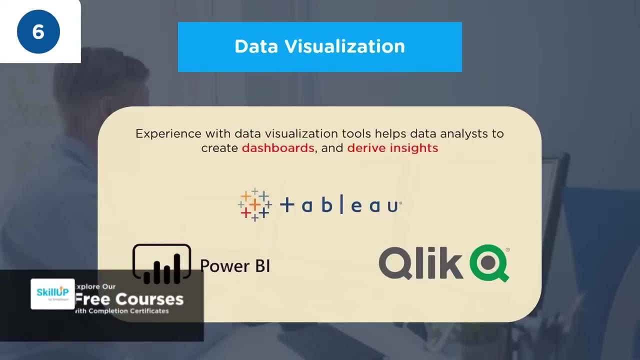 Python and R language provide a collection of different libraries and packages, such as NumPy, Pandas, dplyr, matplotlib, ggplot, which data analysts can use to discover trends and patterns from complex data sets. After this, we have data visualization as our sixth skill. 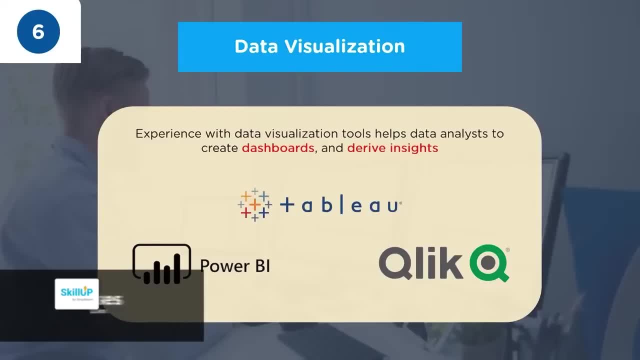 Another data analyst's job role is to visualize large volumes of data and prepare summary reports and dashboards for the leadership team and clients so that they can make timely business decisions. To do this, data analysts use various data visualization tools such as Power BI, Tableau and QlikView. 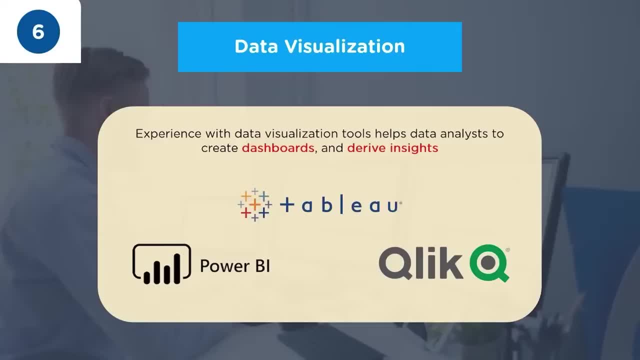 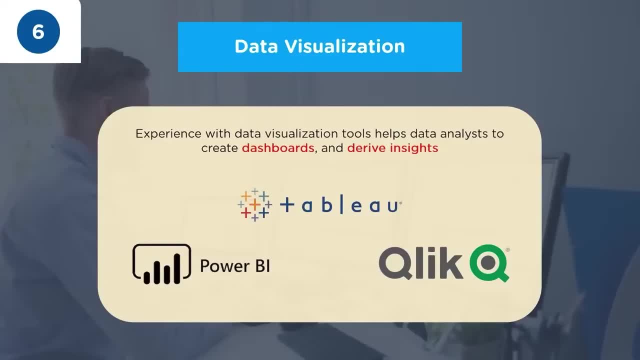 this, data analysts use various data visualization tools, such as power bi, tab blue and click view. using these tools, data analysts can integrate various data sets, apply joint conditions, sort and filter data, as well create different visualizations using charts and graphs. the seventh skill for a data analyst is: 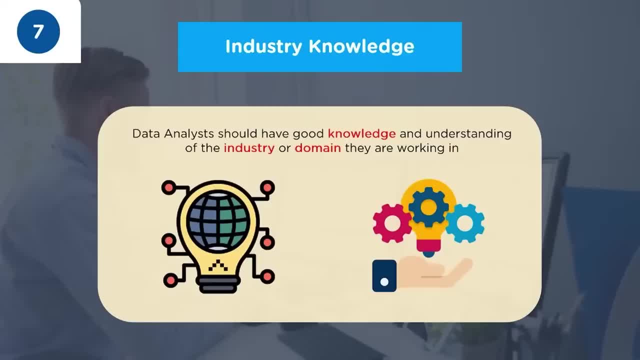 industry knowledge. data analysts should have good knowledge and understanding of the industry or domain they are working in. for example, if you're working in a healthcare domain, you need to know how healthcare analytics can be applied to improve patient care. you should have knowledge about the challenges faced in healthcare and how you can leverage data and analytics to 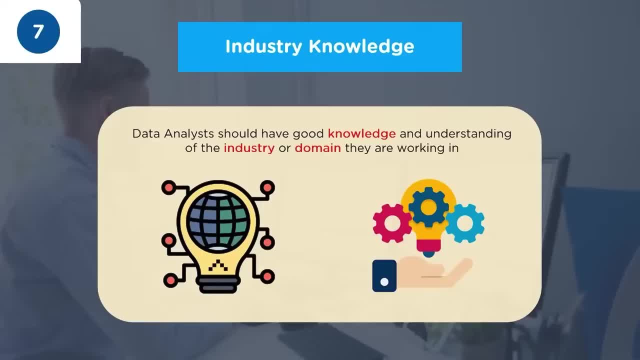 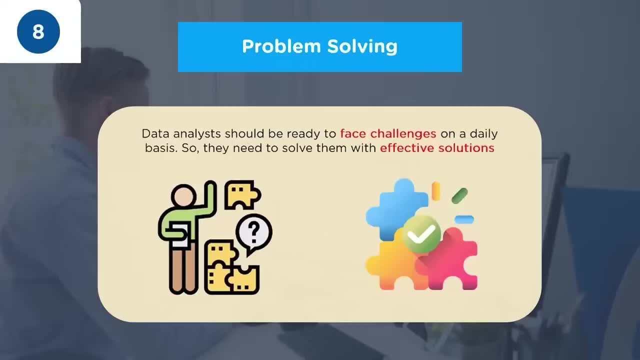 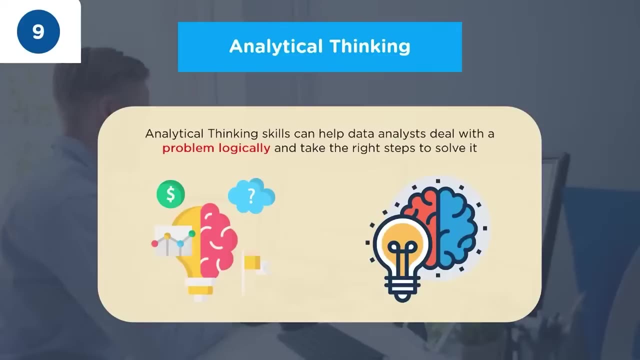 solve the issues. only if you have strong industry knowledge can you try to improve the business. the eighth skill that is important for a data analyst is for a data analyst in 2022- is problem solving. A business deals with several problems on a daily basis. Data analysts should be ready to face those challenges. Data analysts are 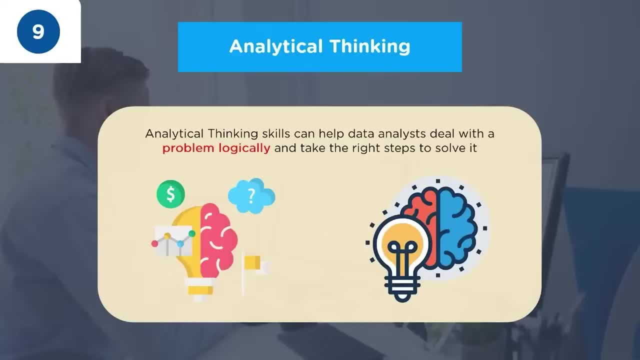 expected to use their problem-solving skills, work with the team, troubleshoot what went wrong and provide an effective solution via data analysis. A data analyst with good problem-solving skills can help a business identify current and potential issues and determine a viable solution based on the data it collects. The ninth skill on our list is Analytical Thinking. 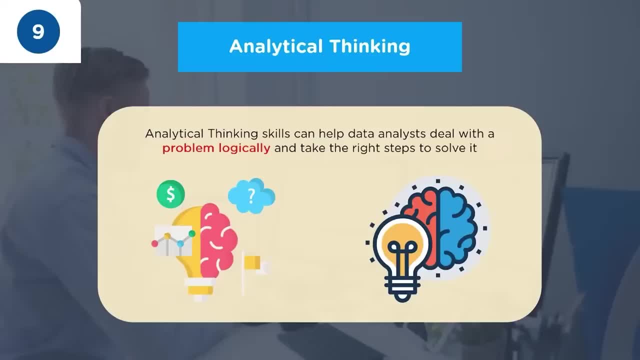 Data analysts need analytical thinking: ability to break down a complex problem into simple components and resolve these components one by one. It is a must-have skill for data analysts. Analytical thinking includes deciding the parameters that need to be considered for defining data sets, analysing them from different perspectives and determining variable. 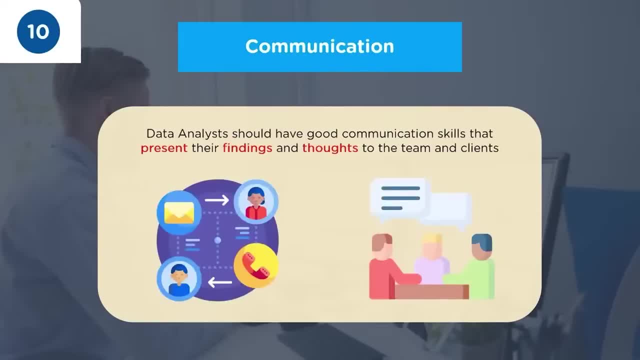 dependencies. Coming to the 10th skill among the top 10 skills for a data analyst in 2022, we have Communication. Data analysts don't just interact with computers and programs. they also interact with team members, stakeholders and data suppliers. So good communication skills. 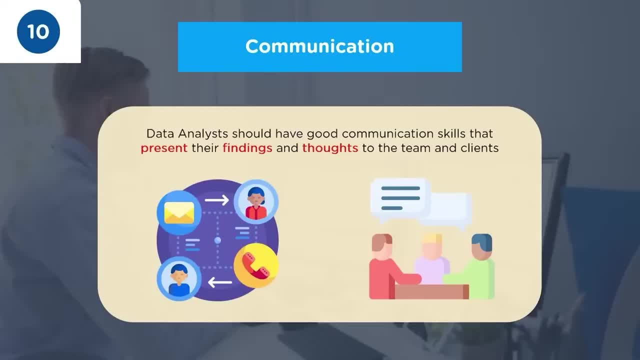 are essential. Data analysts also present their findings in front of an audience who might be interested in learning more about data. Data analysts also present their findings in front of an audience who might not be familiar with the analytical methods and processes, So they need to clearly translate their findings and insights into non-technical terms. 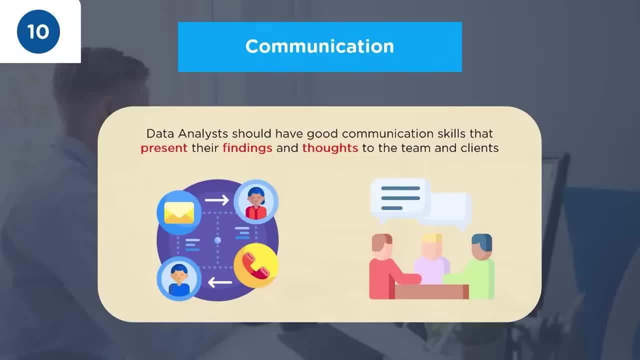 So those were the top 10 skills a data analyst needs to possess in 2022.. Do you think we missed out on any skills? Then please put your answers in the comment section below. Now let's look at the salary of a data analyst According to Glassdoor. 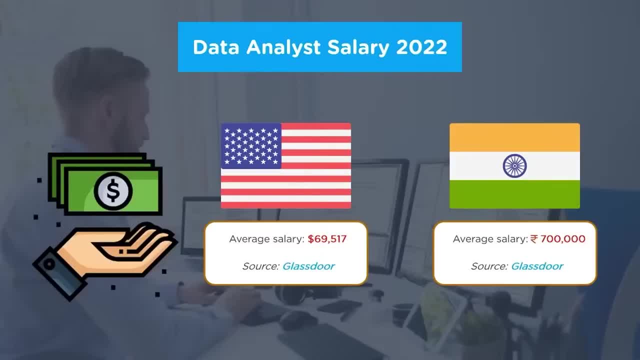 the average annual salary for a data analyst in the United States is $69,500.. While in India, you can earn nearly 7 lakh rupees per annum. Finally, let's look at the top companies that are hiring data analysts in 2022. 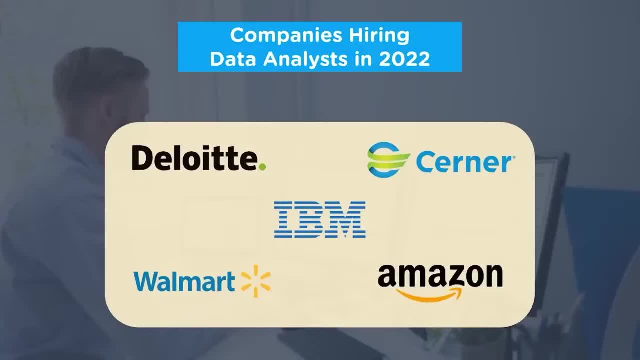 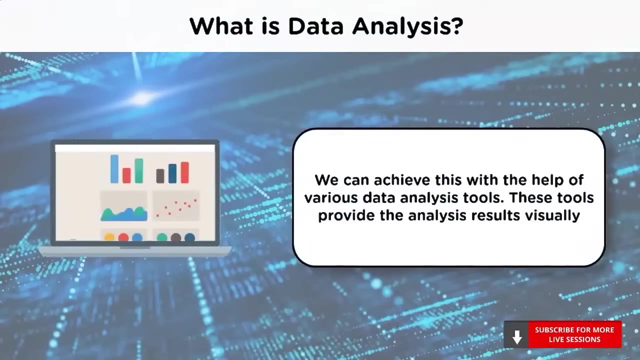 Here we have the consultancy and big four giant, Deloitte and the pharmaceutical company, Cerner Corporation. Then we have the tech giant IBM, retail company Walmart and the e-commerce leader, Amazon. To achieve the goals of data analysis, we use a number of tools, For example: 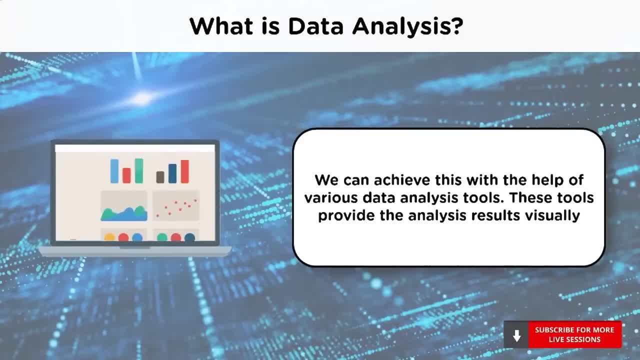 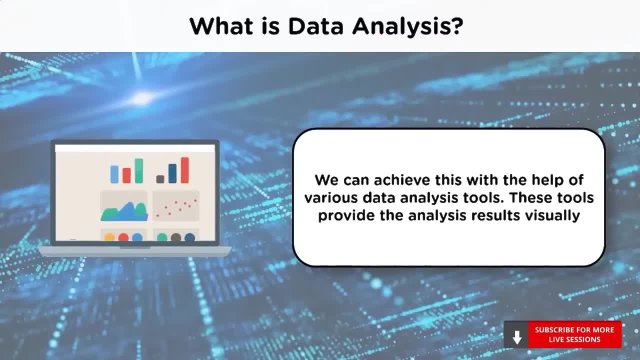 gather and transform their data into meaningful insights. So which tool should you choose to analyze your data? Which tool should you learn if you want to make a career in this field? We will answer that in this session. After extensive research, we have come up with these. 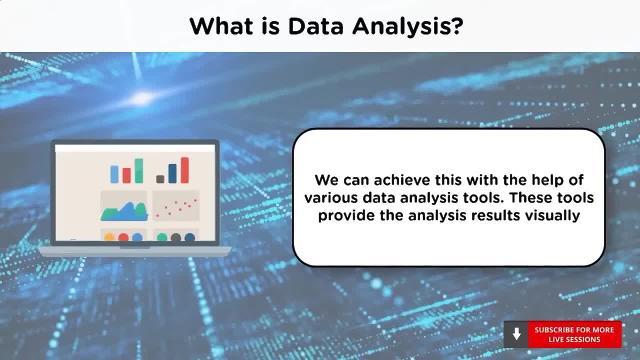 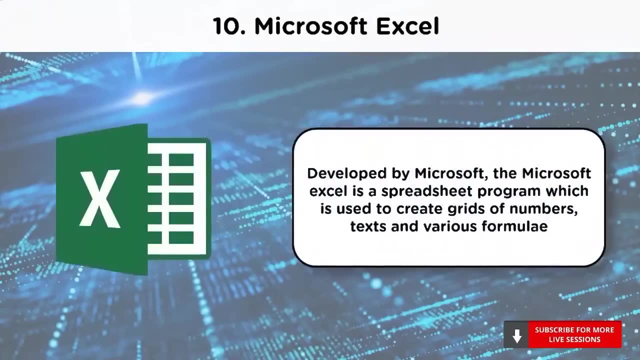 top 10 data analysis tools. Here we will look at the features of each of these tools and the companies using them. So let's start off At number 10, we have Microsoft Excel. All of us would have used Microsoft Excel at some point, right? 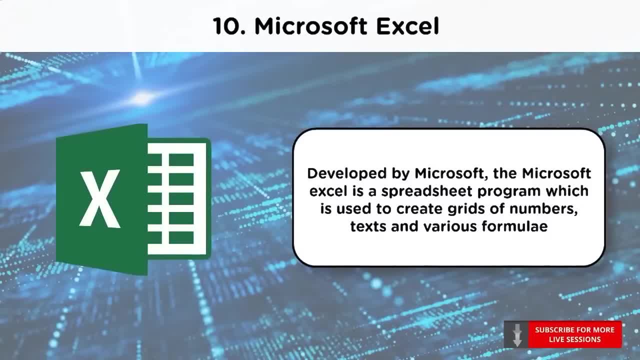 It is easy to use and one of the best tools for data analysis Developed by Microsoft. Excel is basically a spreadsheet program. Using Excel, you can create grids of numbers, text and formulae. It is one of the widely used tools, be it in a small or large setup. 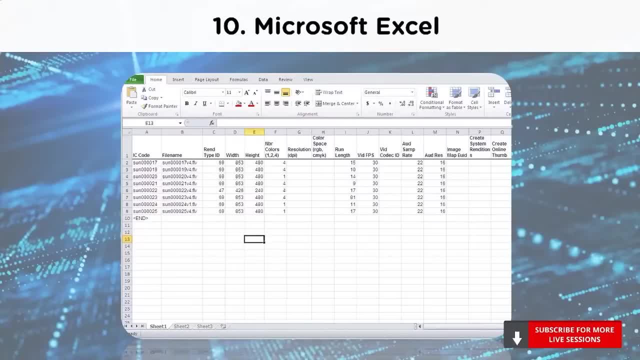 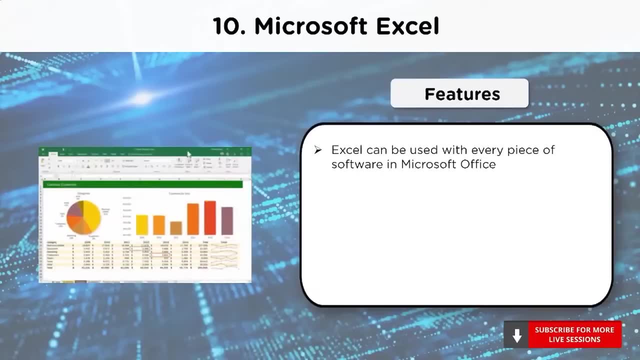 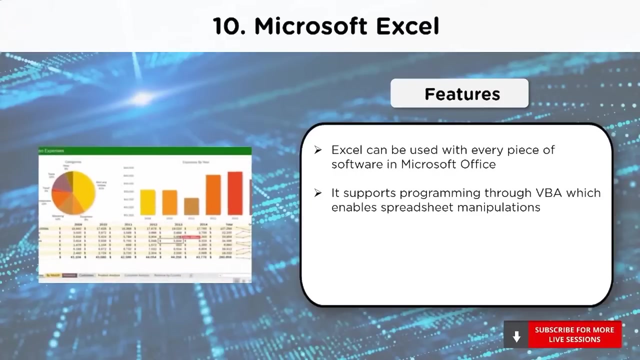 The interface of Microsoft Excel looks like this. Let's now move on to the features of Excel. Firstly, Excel works with Windows. The Windows version of Excel supports programming through Microsoft's Visual Basic for Applications. Programming with VBA allows spreadsheet manipulation that is difficult with standard spreadsheet. 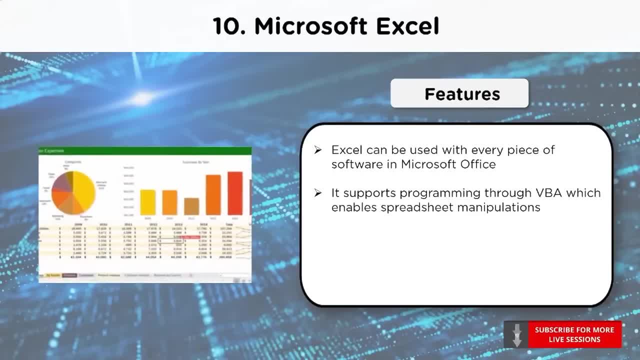 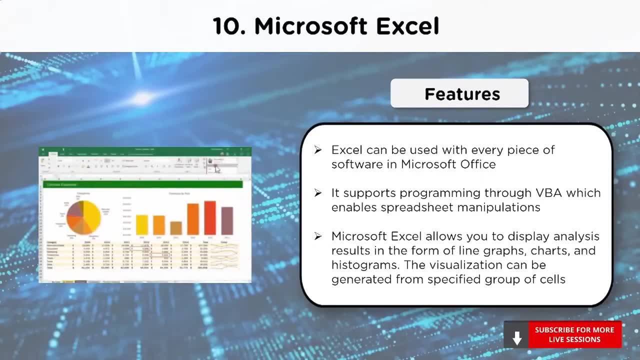 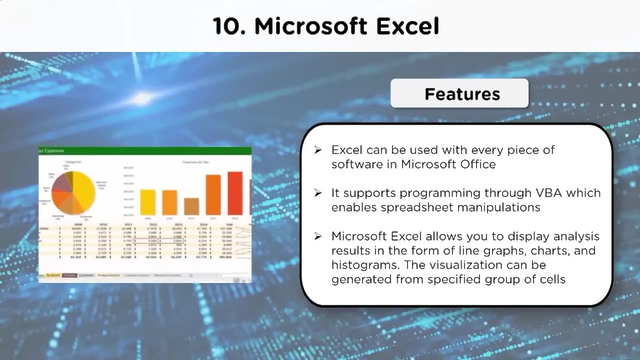 techniques. In addition to this, the user can automate tasks such as formatting or data organization in VBA. One of the biggest benefits of Excel is its ability to organize large amounts of data into orderly, logical spreadsheets and charts. By doing so, it's a lot easier to analyze data, especially while creating graphs and 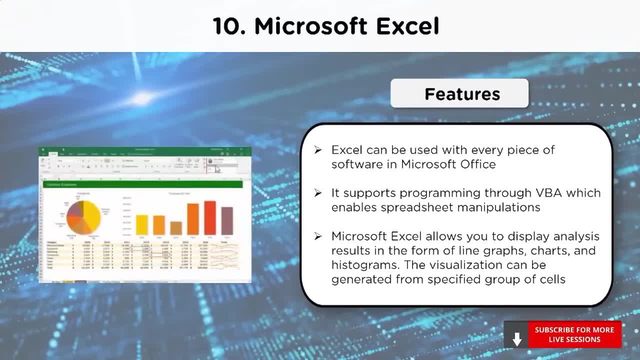 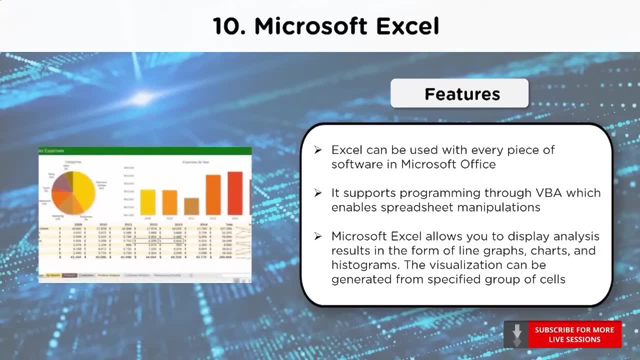 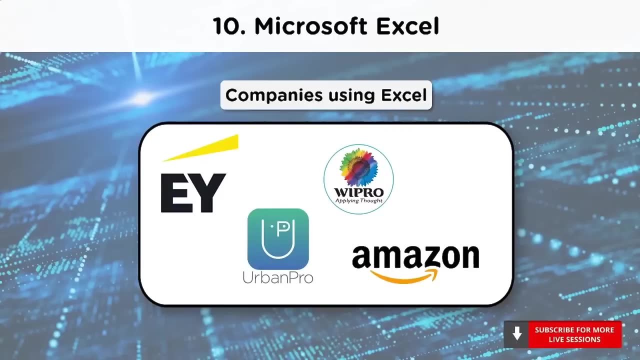 other visual data representations. The visualization can be generated from specified group of cells. Those were few of the features of Microsoft Excel. Let's now have a look at the companies using it. Most of the organizations today use Excel. Few of them that use it for analysis are the UK-based company Ernest & Young. then we 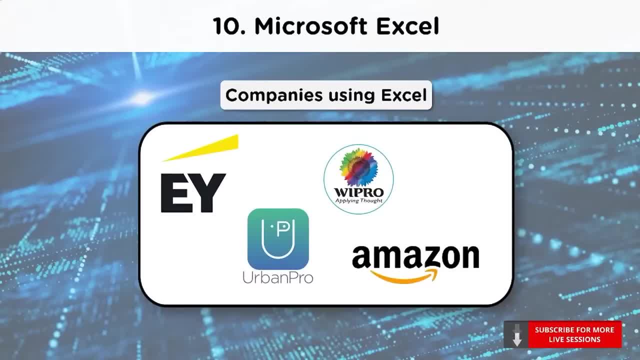 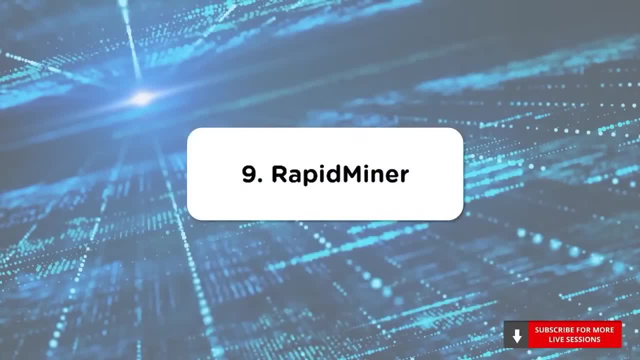 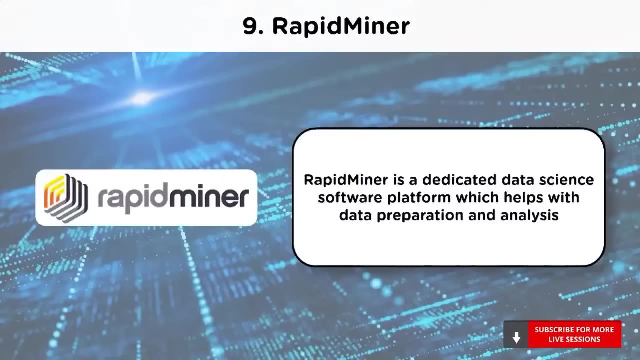 have Urban, Pro, Wipro and Amazon. Moving on to our next data analysis tool, at number 9, we have RapidMiner, A data science software platform. RapidMiner provides an integrated environment for data preparation, analysis, machine learning and deep learning. 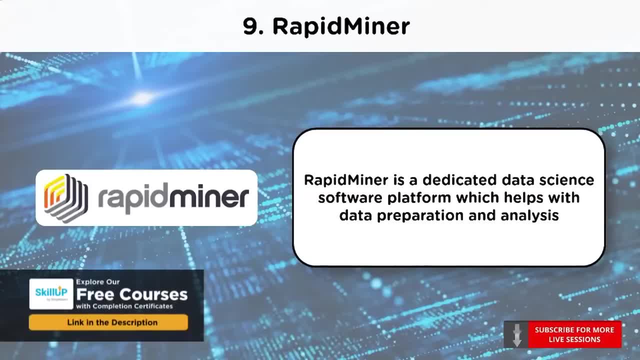 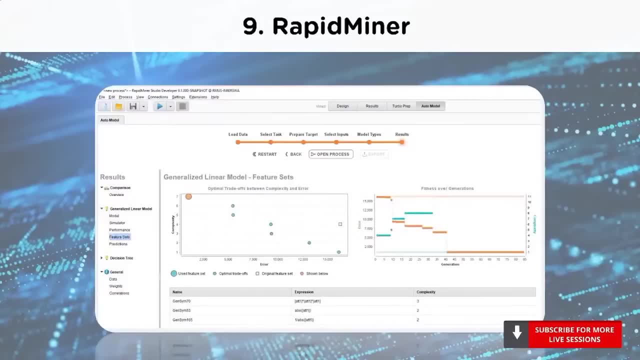 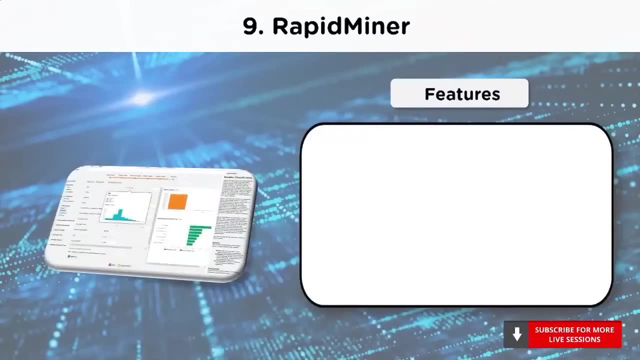 It is used in almost every business and commercial sector. RapidMiner also supports all the steps of the machine learning process. Seen on your screens is the interface of RapidMiner. Moving on to the features of RapidMiner, Firstly, it offers the ability to drag and drop. 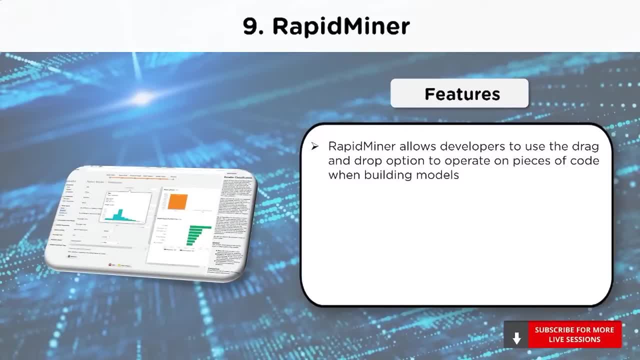 It is very convenient to just drag-drop some columns as you are exploring a data set and working on some analysis. RapidMiner allows you to drag and drop some columns as you are exploring a data set and working on some analysis. RapidMiner allows you to drag and drop some columns. 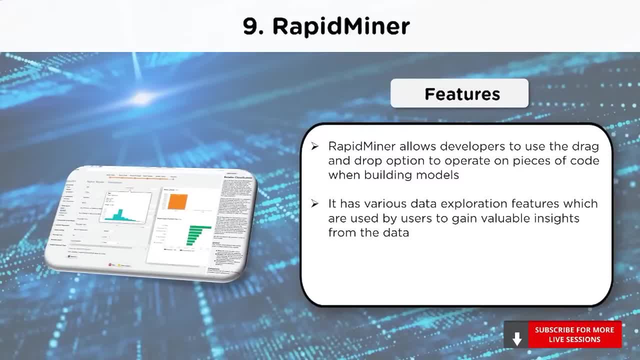 It allows the usage of any data and it also gives an opportunity to create models which are used as a basis for decision making and formulation of strategies. It has data exploration features such as graphs, descriptive statistics and visualization, which allows users to get valuable insights. 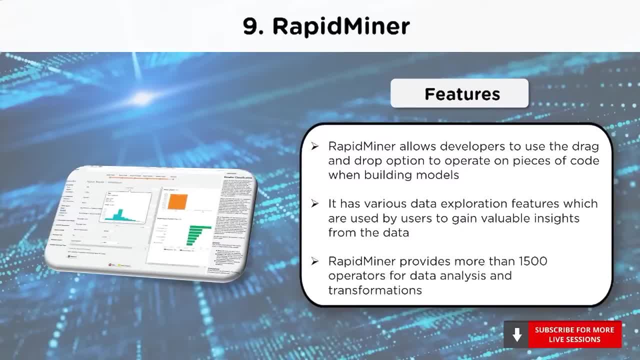 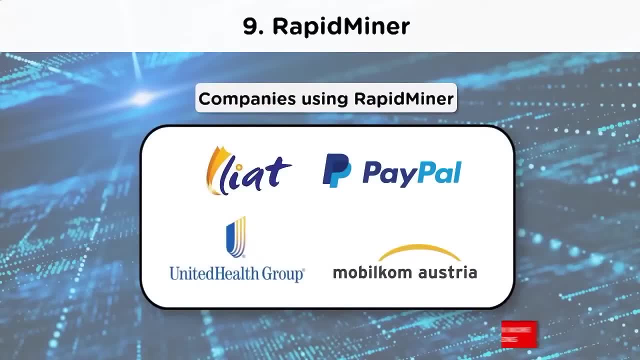 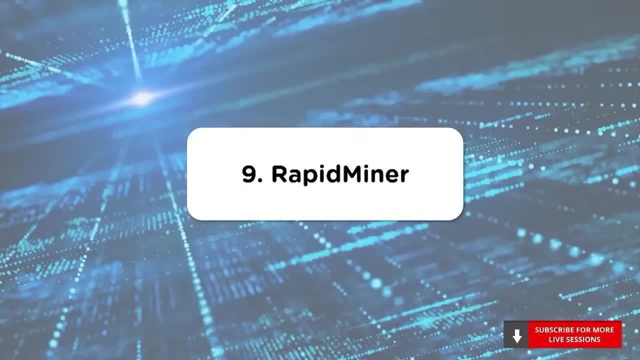 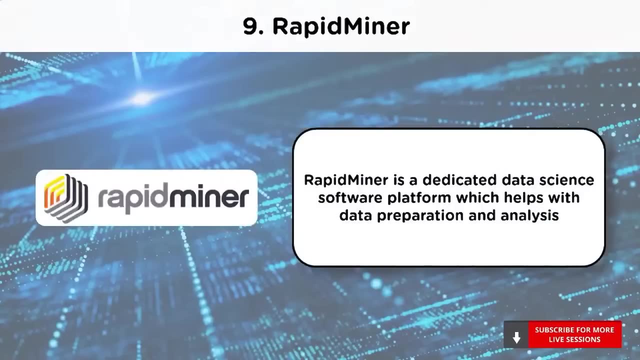 Data analysts need analytical thinking ability to break down a complex problem into simple components, one by one. Moving on to our next data analysis tool, at number 9 we have RapidMiner, A data science software platform. RapidMiner provides an integrated environment for data. 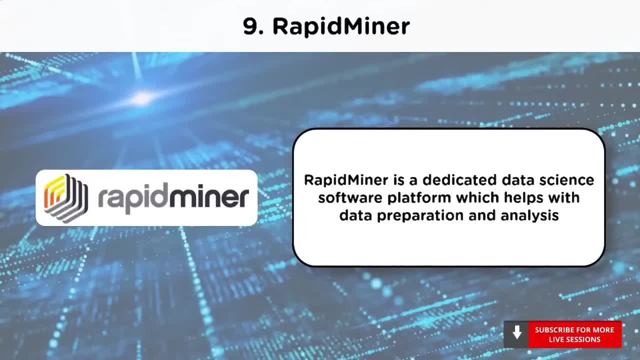 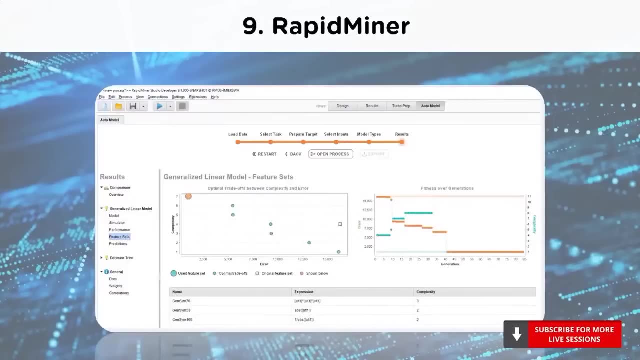 preparation, analysis, machine learning and deep learning. It is used in almost every business and commercial sector. RapidMiner also supports all the steps of the machine learning process. Seen on your screens is the interface of RapidMiner. Moving on to the features of RapidMiner, 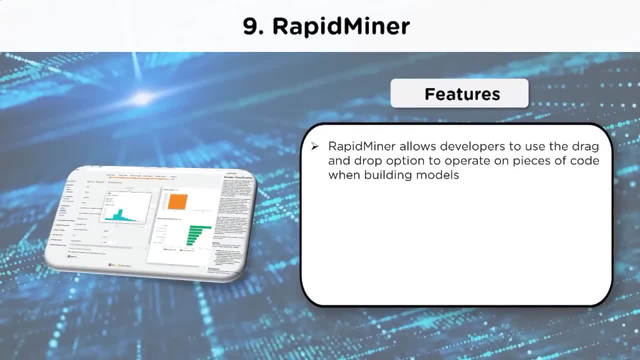 Firstly, it offers the ability to drag and drop. It is very convenient to just drag drop some columns as you are exploring a data set and working on some analysis. RapidMiner allows the usage of any data and it also gives an opportunity to create models. 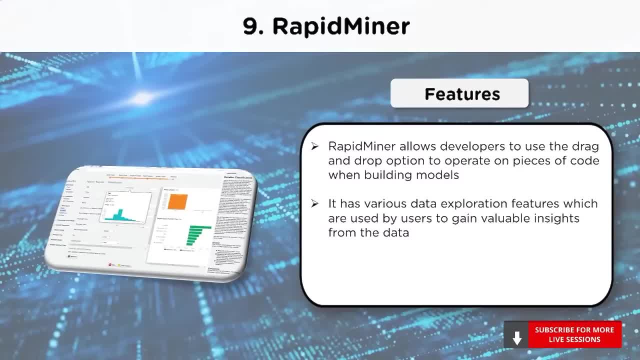 which are used as a basis for decision making and formulation of strategies. It has data exploration features such as graphs, descriptive status statistics and visualization, which allows users to get valuable insights. It also has more than 1,500 operators for every data transformation and analysis task. 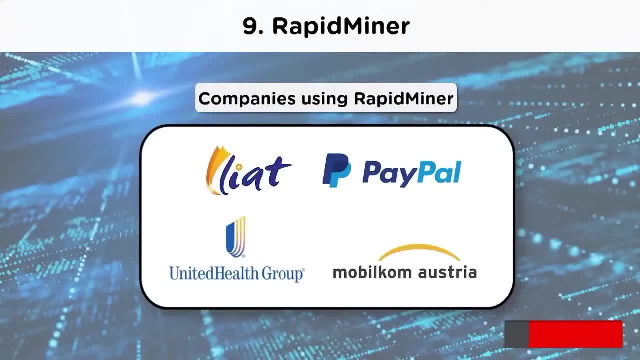 Let's now have a look at the companies using RapidMiner. We have the Caribbean airline, Leeward Islands Air Transport. Next we have the United Health Group, the American online payment company, PayPal, and the Austrian telecom company Mobilcom. So that was all about RapidMiner. 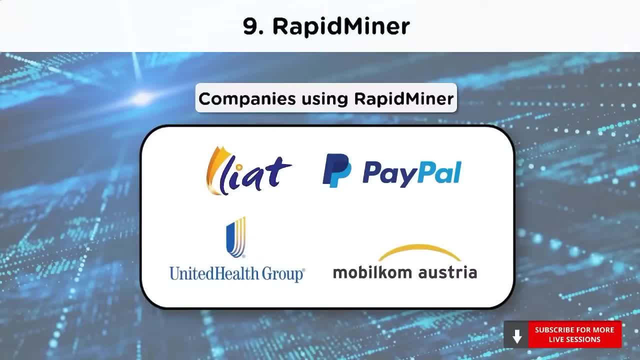 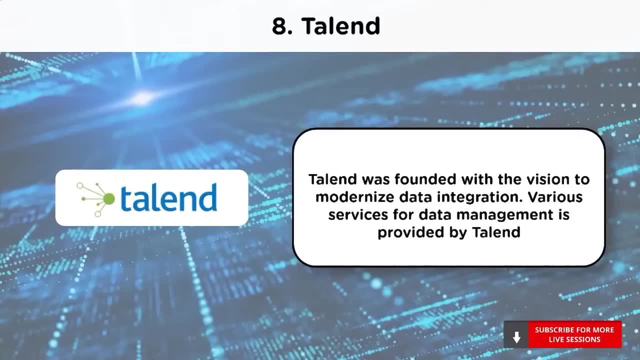 Now let's see which tool we have at number 8.. We have Talent at number 8.. Talent is an open source software platform which offers data integration and management. It specializes in big data integration. Talent is available both in open source and premium versions. 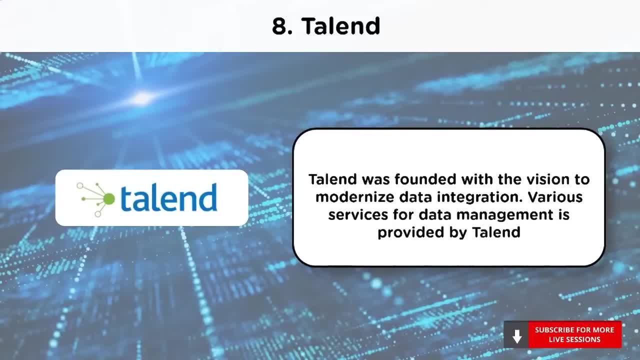 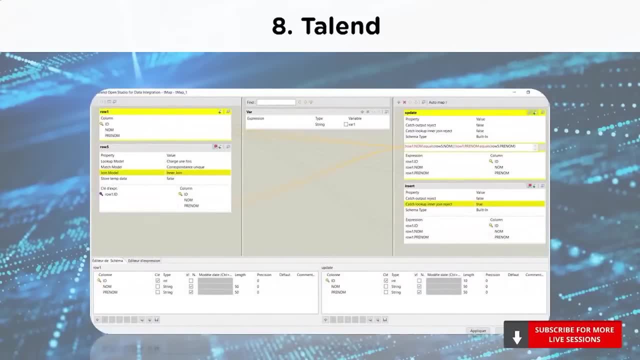 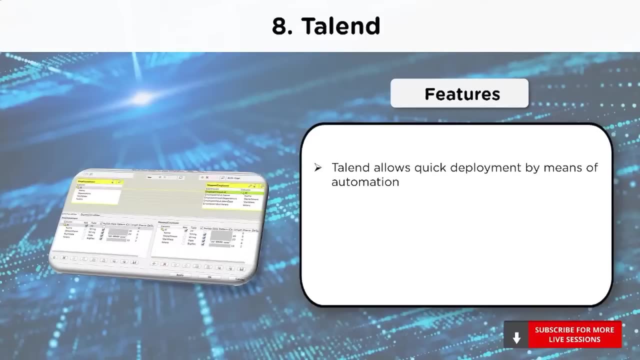 It is one of the best tools for cloud computing and big data integration. The interface of Talent is as seen on your screens. Moving on to the features of Talent, Firstly, automation is one of the great boons Talent offers. It even maintains the tasks for the users. 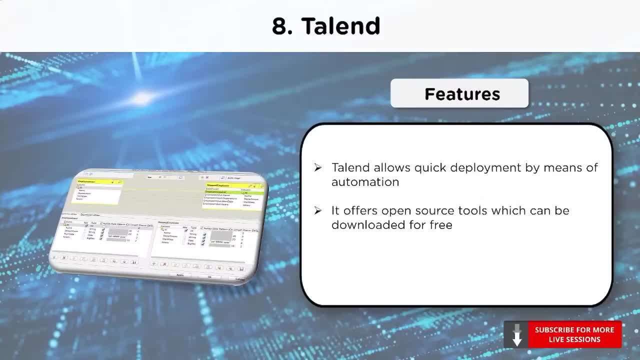 This helps with quick deployment and development. It also offers open source tools. Talent lets you download these tools for free. The development costs reduce significantly as the processes gradually speed up. Talent provides a unified platform. It allows you to integrate with many different applications. 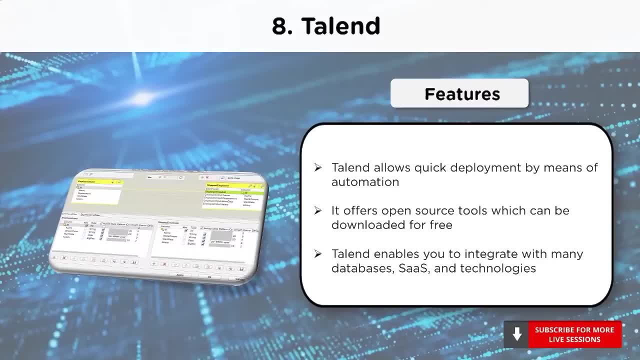 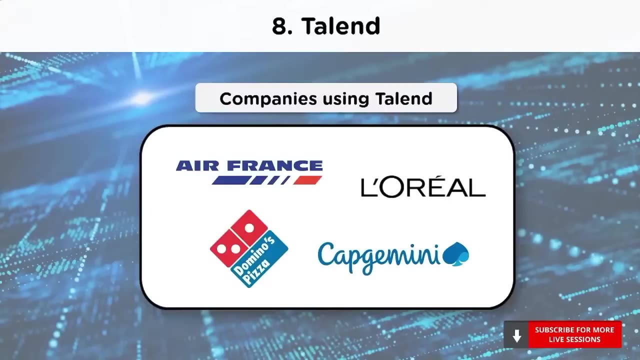 Many databases, SaaS and other technologies. With the help of the data integration platform, you can build flat files, relational databases and cloud apps 10 times faster. Those were the features of Talent. The companies using Talent are Air France, L'Oreal, Capgemini and the American multinational. 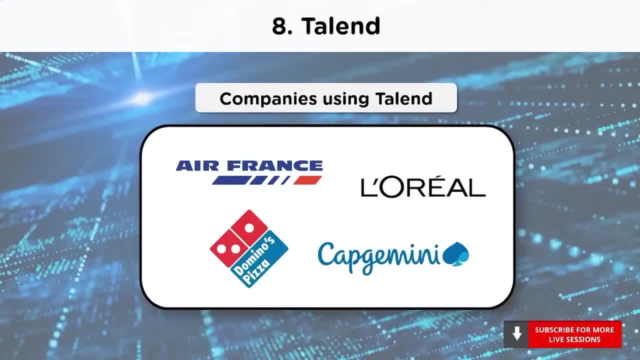 pizza restaurant chain. Domino's Next on the list, at 7, we have 9.. Constance International is one of the most popular companies in the world. It is one of the most popular companies in the world. It is one of the most popular companies in the world. 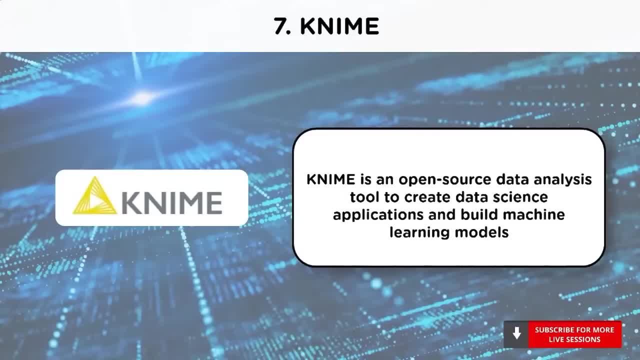 Our information miner, or KNIME, is a free and open source data analytics, reporting and integration platform. It can integrate various components for machine learning and data mining through its modular data pipelining concept. KNIME has been used in pharmaceutical research and other areas like CRM, Customer Data Analysis. 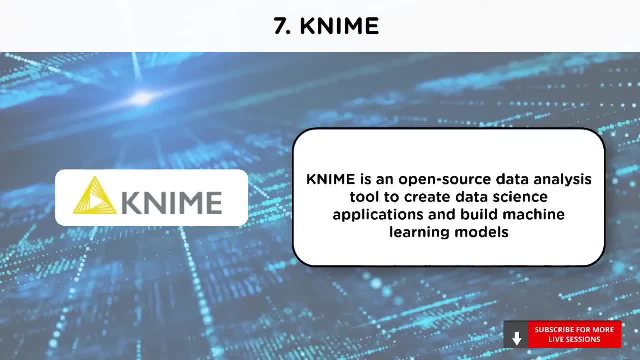 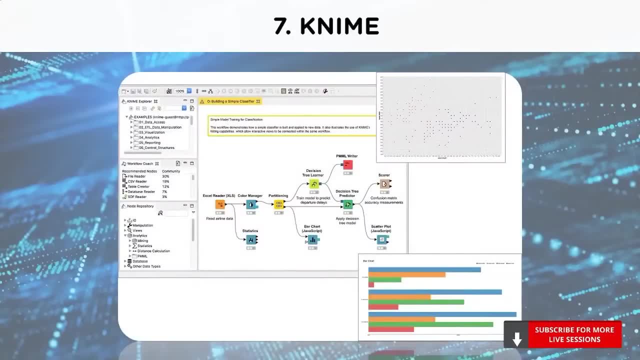 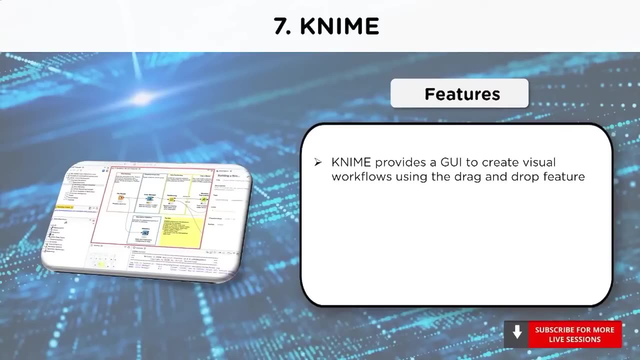 Business Intelligence, Text Mining and Financial Data Analysis. Here is how the interface of KNIME application looks like. We are now going to see how the interface of KNIME application looks like. Now, coming to the KNIME features. KNIME provides an interactive graphical user interface to 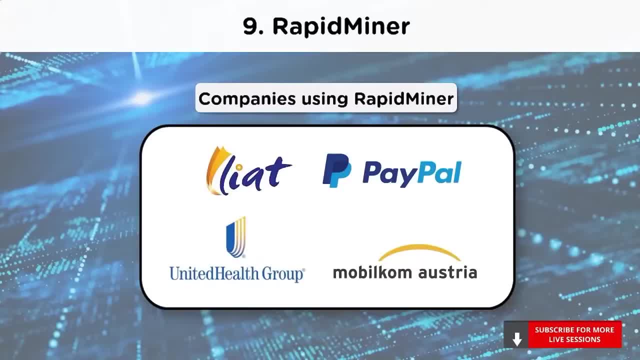 Next we have the United Health Group, the American online payment company PayPal and the Austrian telecom company Mobilecom. So that was all about RapidMiner. Now let's see which tool we have at number 8.. We have Talent at number 8.. 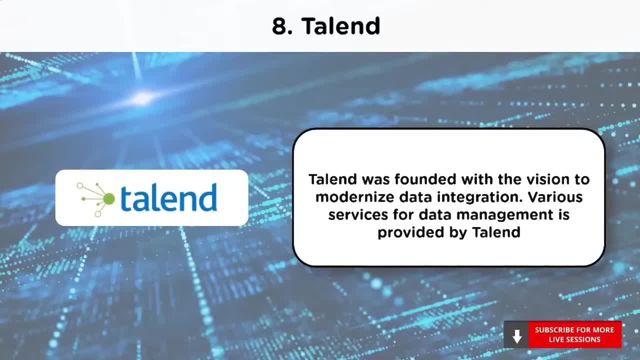 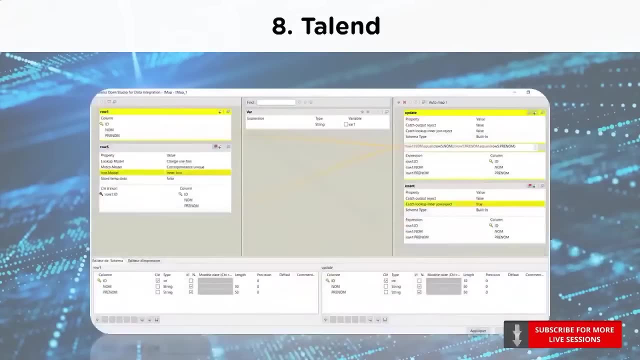 Talent is an open source software platform which offers data integration and management. It specializes in big data integration. Talent is available in many languages. Talent is available both in open source and premium versions. It is one of the best tools for cloud computing and big data integration. 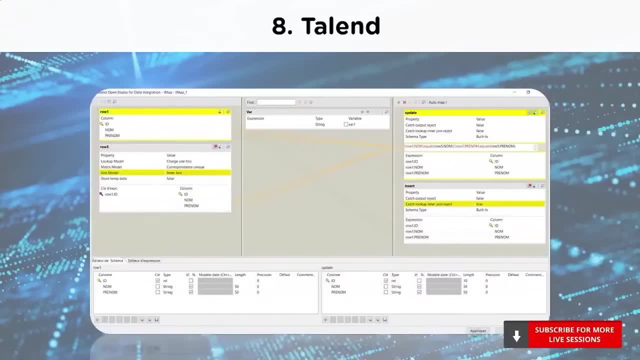 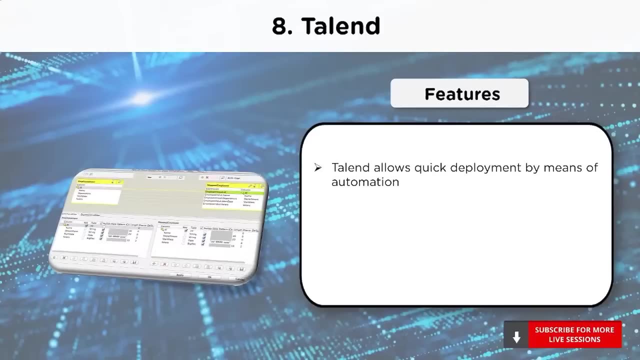 The interface of Talent is as seen on your screens. Moving on to the features of Talent, Firstly, Automation is one of the great boons Talent offers. It even maintains the tasks for the users. This helps with quick deployment and development. It also offers automatic automation. 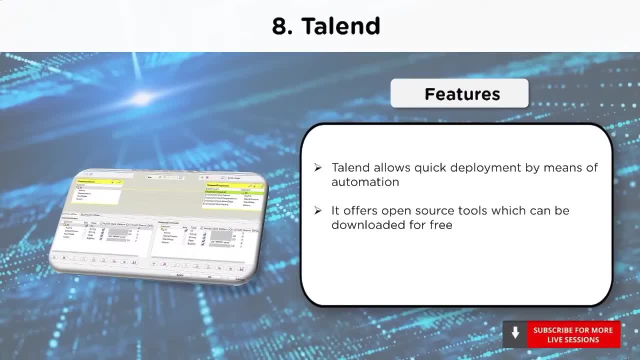 It also offers automatic automation. It also offers open source tools. Talent lets you download these tools for free. The development costs reduce significantly as the processes gradually speed up. Talent provides a unified platform. It allows you to integrate with many databases, SaaS and other technologies. 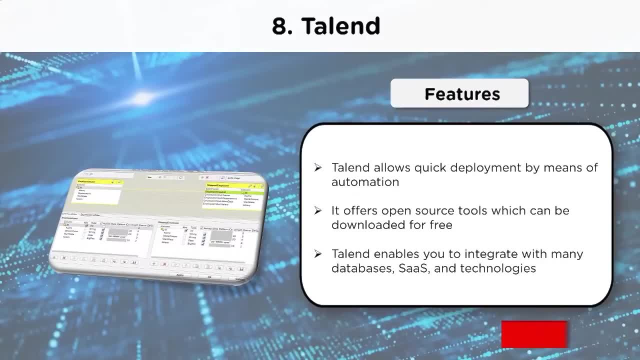 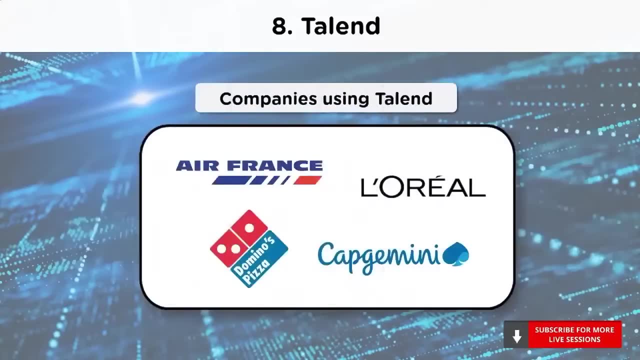 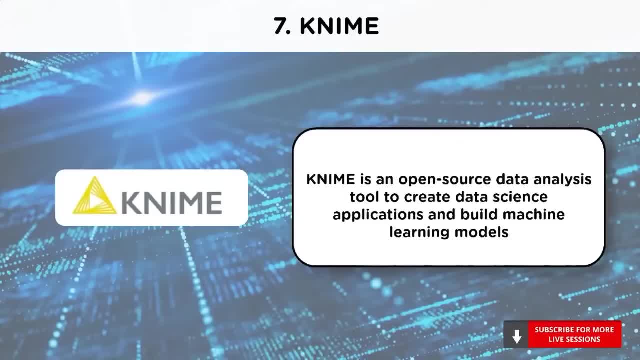 Next on the list, at 7, we have KNIME. Constance Information Miner, or KNIME, is a free and open source data analytics reporting and integration platform. It can integrate various components for machine learning and data mining through its modular data pipelining concept. 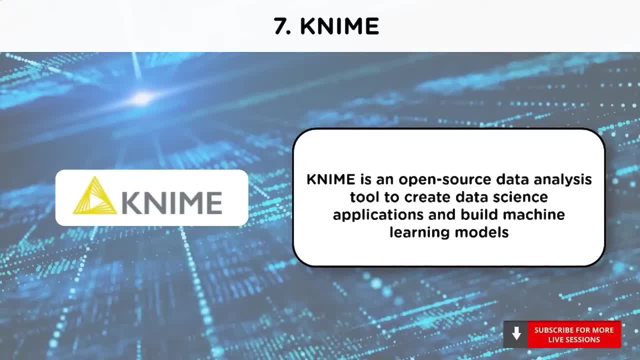 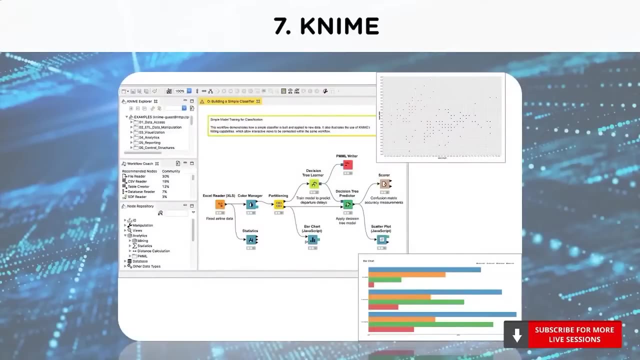 KNIME has been used in pharmaceutical research and other areas like CRM, customer data analysis, business intelligence, text mining and financial data analysis. Here is how the interface of KNIME application looks like. Now, coming to the KNIME features. KNIME provides an interactive graphical user interface to 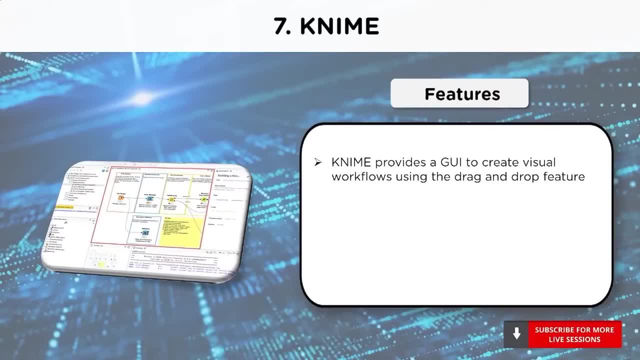 create visual workflows using the drag-and-drop feature. Use of JDBC allows assembly of nodes blending different data sources, including preprocessing, such as ETL for modeling, data analysis and visualization, with minimal programming. It supports multi-threaded in-memory data processing. 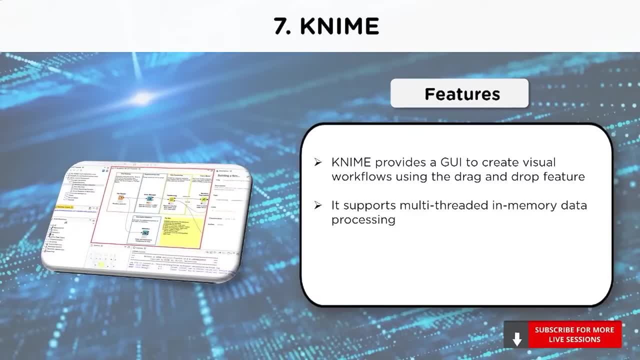 KNIME allows users to visually create data flows, selectively execute some or all analysis steps and later inspect the results, models and interactive views. KNIME Server automates workflow execution and supports team-based collaboration. KNIME integrates various other open-source projects, such as machine learning algorithms. 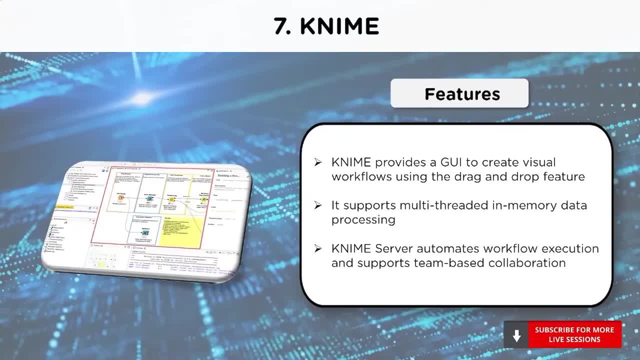 from Beka, H2O, Keras, Spark and our project KNIME allows analysis of the data flow and integrates the data flow into the data processing process. KNIME has a large database of 300 million custom addresses, 20 million cell images. 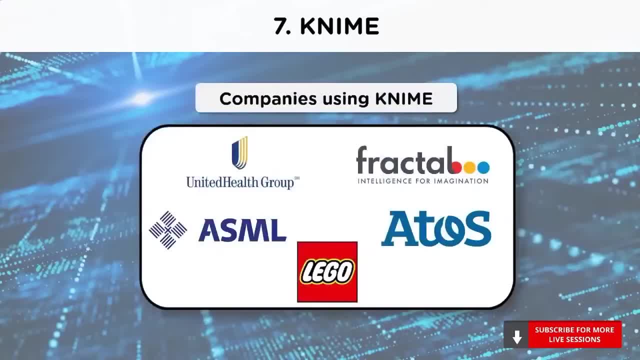 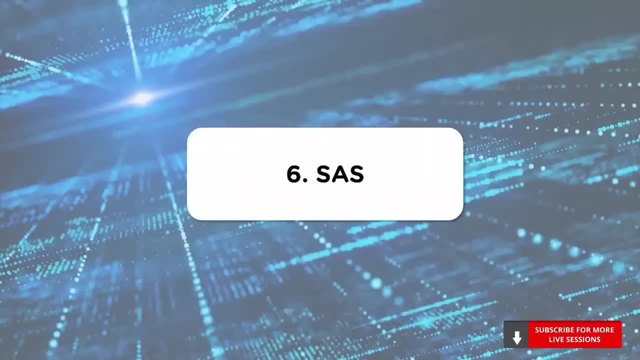 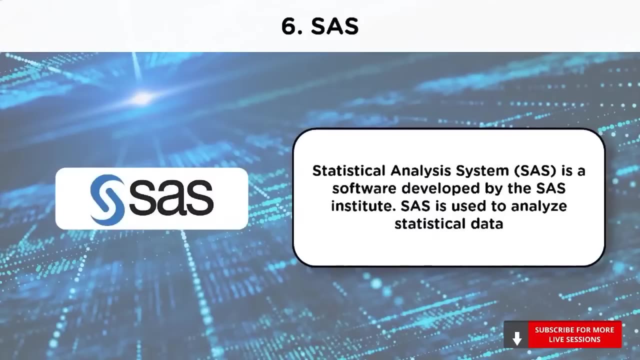 and 10 million molecular structures. Some of the companies hiring for KNIME are United Health Group, ASML, Fractal Analytics, Atos and Lego Group. Let's now move on to the next tool. We have SAS at number 6.. 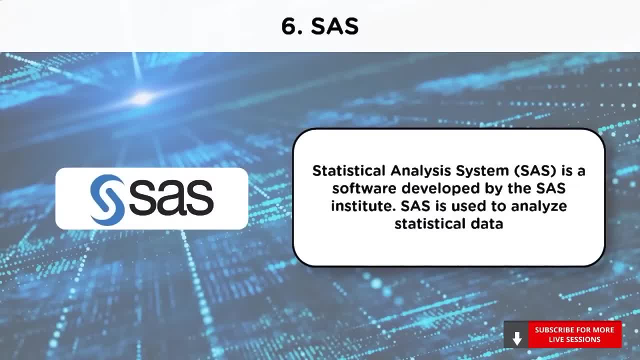 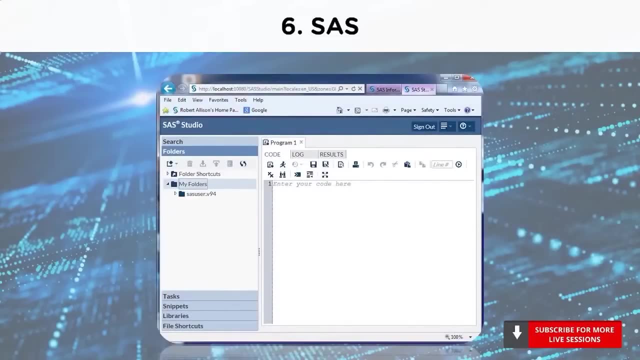 SAS facilitates analysis, reporting and predictive modeling with the help of powerful visualizations and dashboards. In SAS, data is extracted from the data source. The data is extracted and categorized, which helps in identifying and analyzing data patterns. As you can see on your screens, this is how the interface looks like. 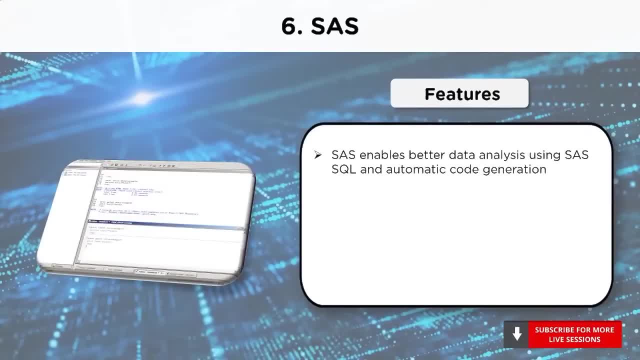 Moving on to the features of SAS, Using SAS, better analysis of data is achieved by using automatic code generation and SAS SQL. SAS allows you to access through Microsoft Office by letting you create reports using it and by distributing them through it. SAS allows you to access through Microsoft Office by letting you create reports using it and by distributing them through it. 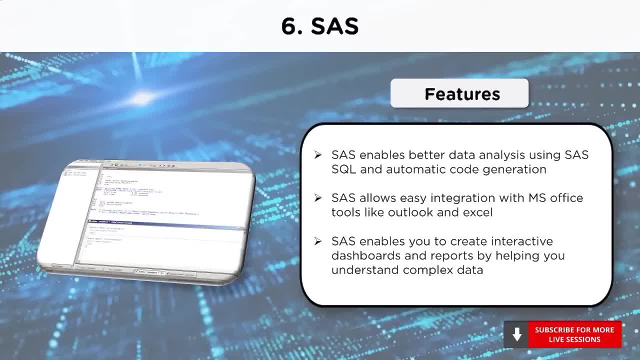 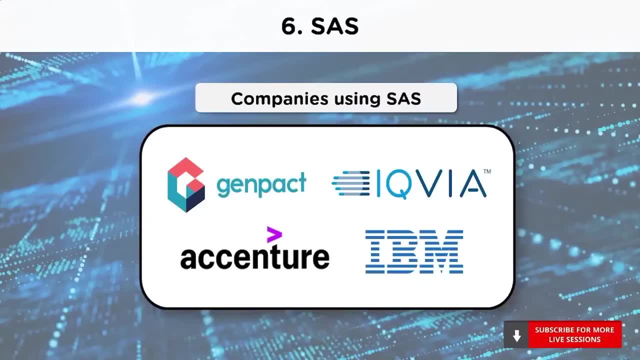 SAS helps with an easy understanding of complex data and allows you to create interactive dashboards and reports. Let's now have a look at the companies using SAS. We have companies like Genpak, IQVR, Accenture and IBM, to name a few. 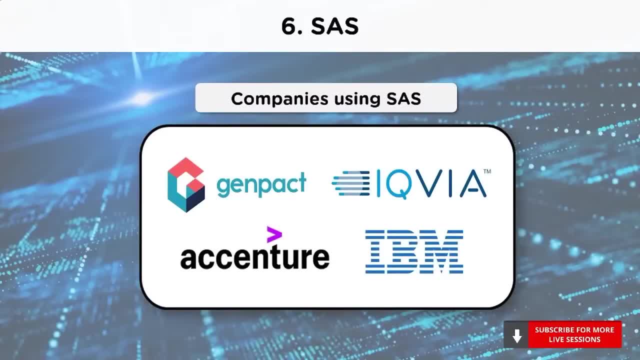 That was all about SAS. So for all those who joined in late, let me just quickly repeat our list: At number 10, we have Microsoft Excel, Then at number 9, we have RapidMiner, Then at number 10, we have Microsoft Excel. 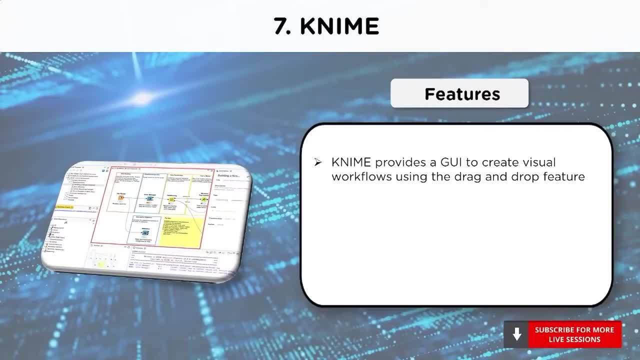 create visual workflows using the drag and drop feature. Use of JDBC allows assembly of nodes blending different data sources, including pre-processing, such as ETL for modeling, data analysis and visualization, with minimal programming. It supports multi-threaded in-memory data processing. 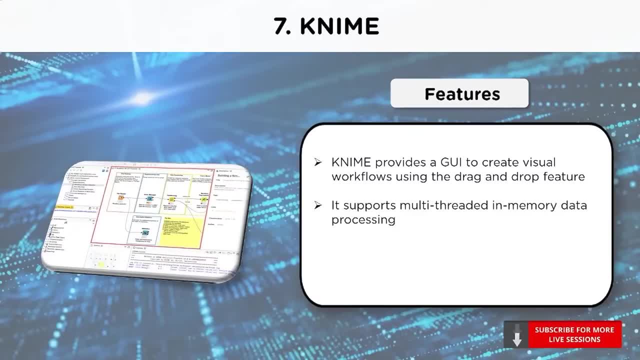 KNIME allows users to visually create data flows, selectively execute some or all analysis steps and later inspect the results, models and interactive views. KNIME Server- Automatic Data Processing. KNIME estimates workflow execution and supports team-based collaboration. KNIME integrates various other open-source projects, such as machine learning algorithms. 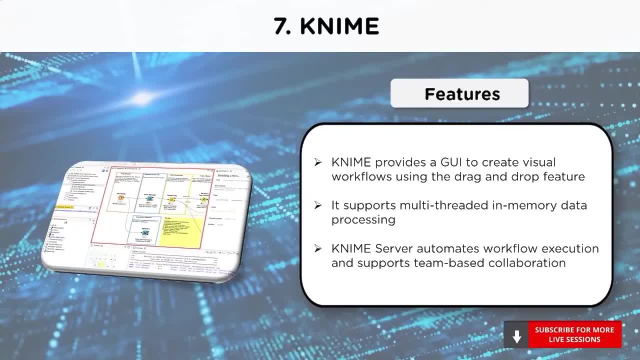 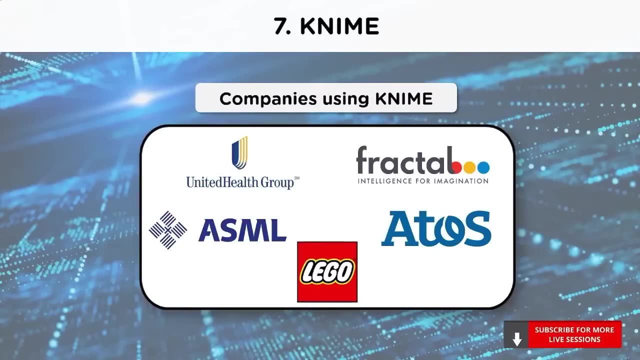 from Beka, H2O, Keras Park and our project, KNIME, allows analysis of 300 million custom addresses, 20 million cell images and 10 million molecular structures. Some of the companies hiring for KNIME are United Health Group, ASML, Fractal Analytics. 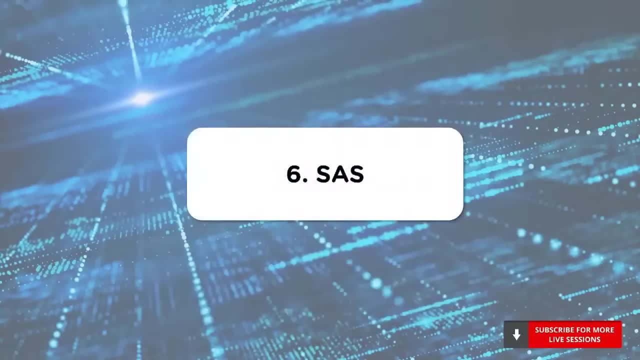 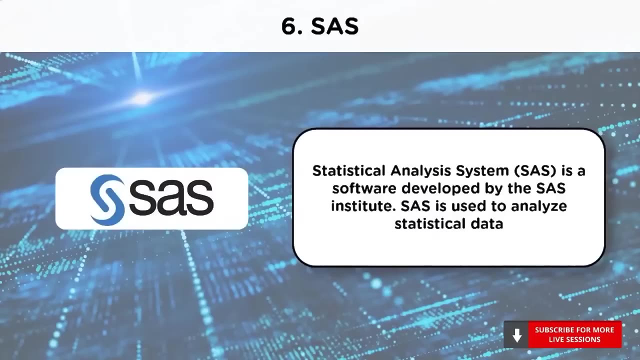 Atos and Lego Group. Let's now move on to the next tool. We have SAS at number 6.. SAS facilitates analysis, reporting and predictive modeling with the help of powerful visualizations and dashboards. In SAS, data is extracted and categorized, which helps in identifying and analyzing data. 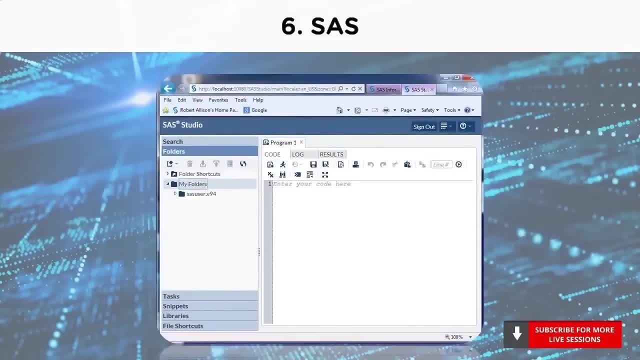 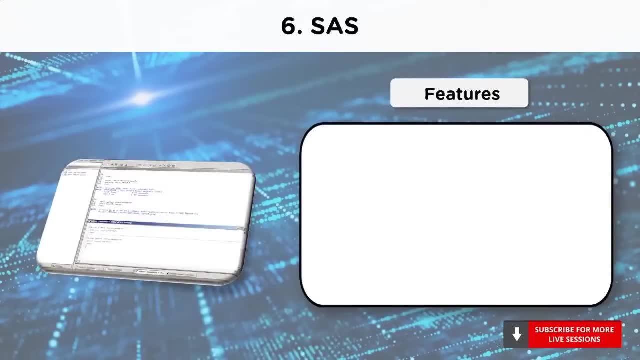 patterns, As you can see on your screens. this is how the interface looks like. Moving on to the features of SAS, Using SAS, better analysis of data is achieved by using automatic code generation and SAS SQL. SAS allows you to access through Microsoft Office by letting you create reports using 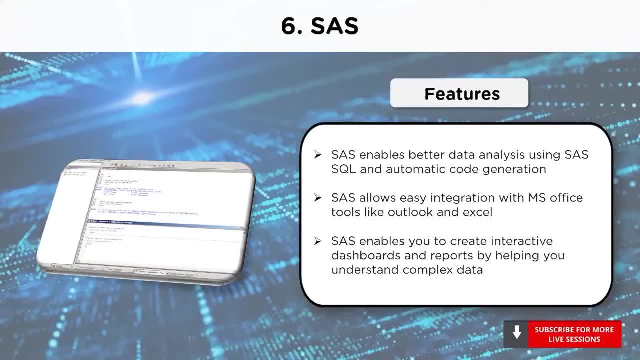 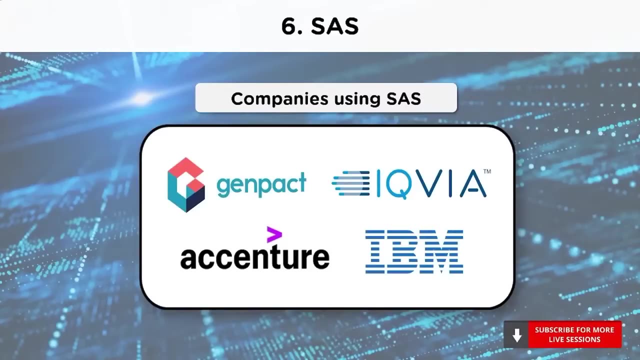 it and by distributing them. through it, SAS helps with an easy understanding of complex data and allows you to create interactive dashboards and reports. Let's now have a look at the companies using SAS. We have companies like Genpakcom, IQVRcom. 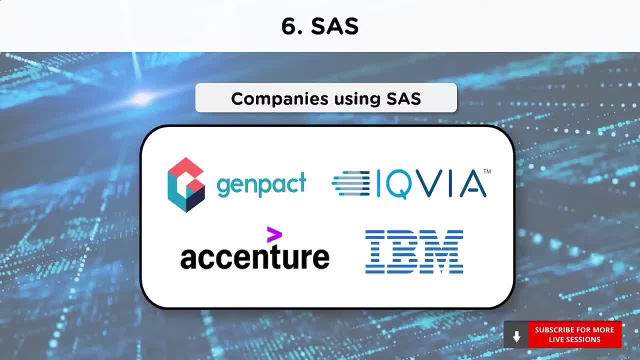 Accenture and IBM, to name a few. That was all about SaaS. So for all those who joined in late, let me just quickly repeat our list. At number 10 we have Microsoft Excel, then at number 9 we have RapidMiner. at number 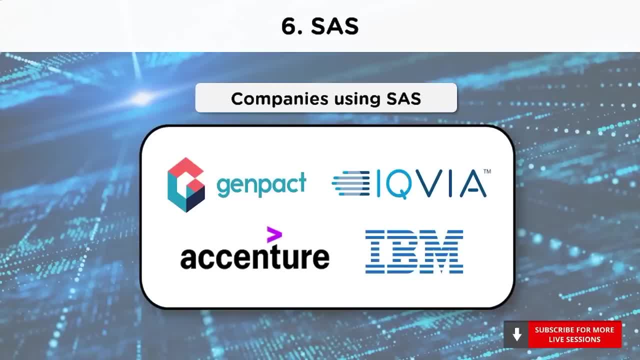 At number 8, we have Talent, At number 7, we have KNIME And at number 6, we have SAS. So far, do you all agree with this list? Let us know in the comment section below. Let's now move on to the next 5 tools in our list. 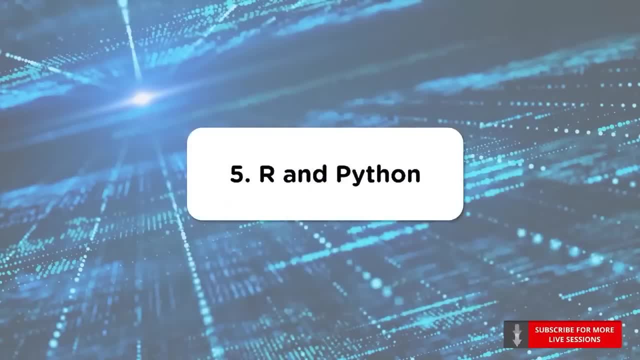 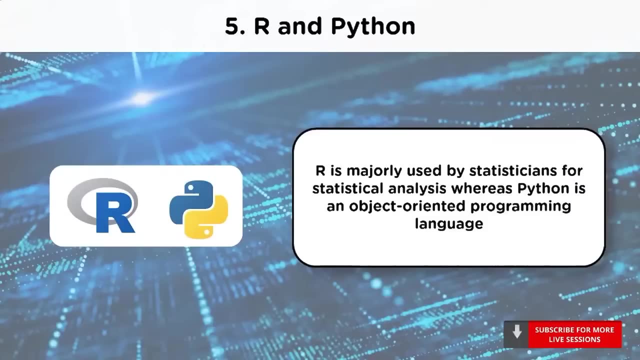 So at number 5, we have both R and Python. Yes, we have two of them. in the 5th position, R is a programming language. R is a programming language which is used for analysis as well. It has traditionally been used in academics and research. 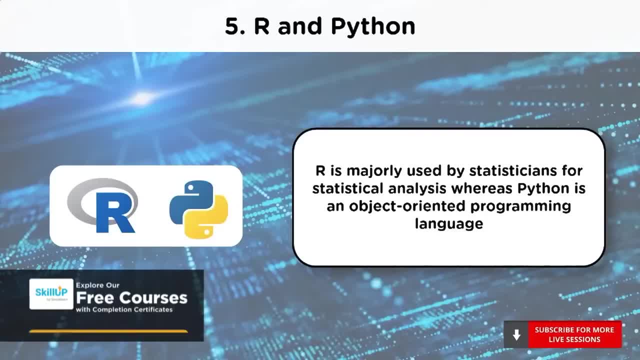 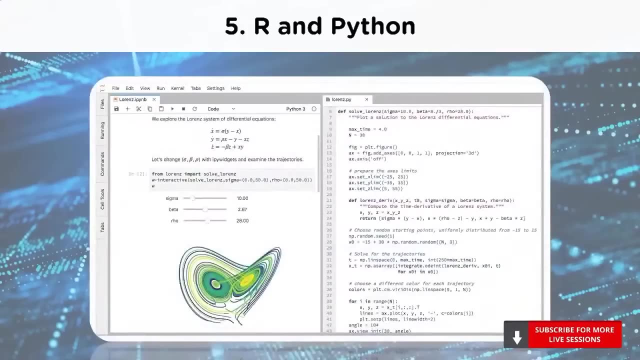 Python is a high-level programming language which has a Python data analysis library. It is used for everything, starting from importing data from Excel spreadsheets to processing them for analysis. This is the interface of R. Next up is the interface of the Python Jupyter. 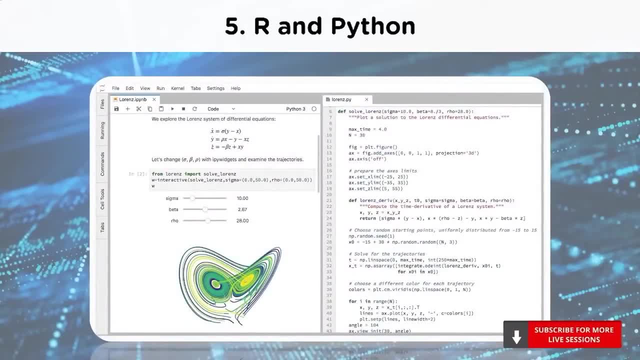 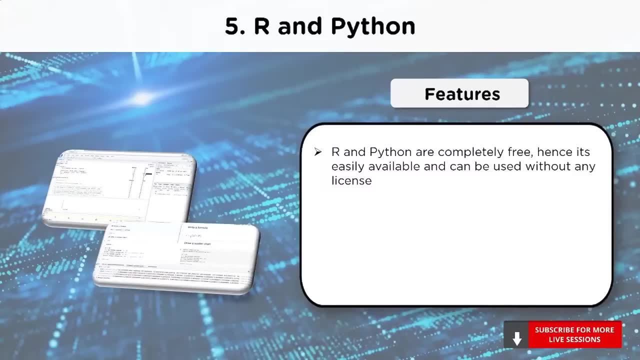 Notebook. Let's now move on to the features of both R and Python. When it comes to the availability of R and Python, it is very easy. Both R and Python are completely free, hence it can be used without any license. R used to compute everything in memory, and hence the computations were limited. but now 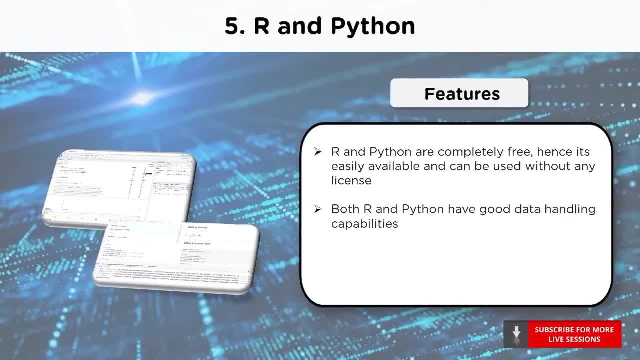 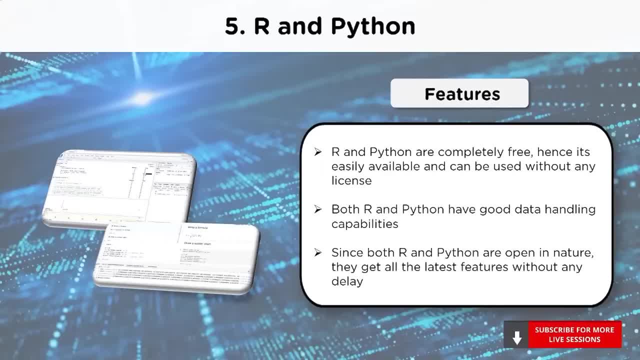 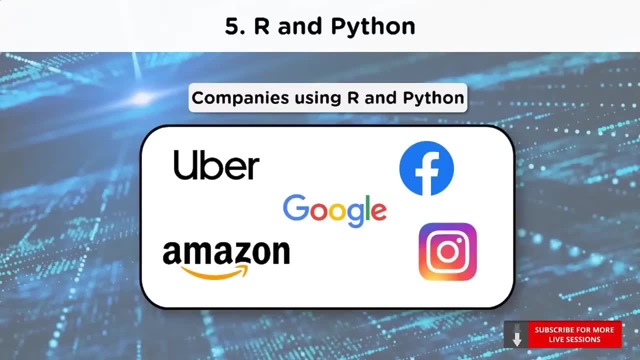 R and Python are compatible. R and Python are open in nature. All the latest features are available without any delay. Moving on to the companies using R, We have Uber, Google, Facebook, to name a few. Python is used by many companies. 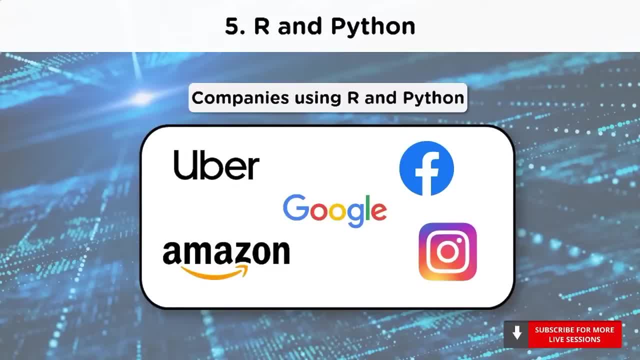 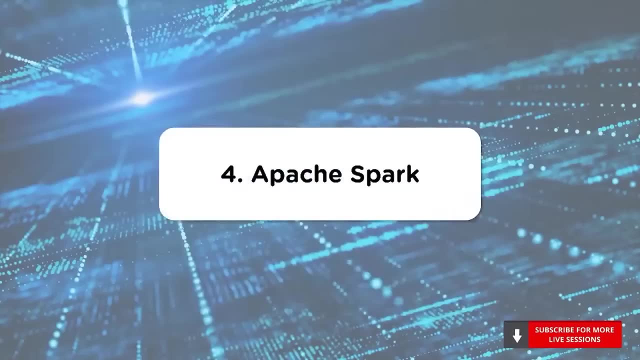 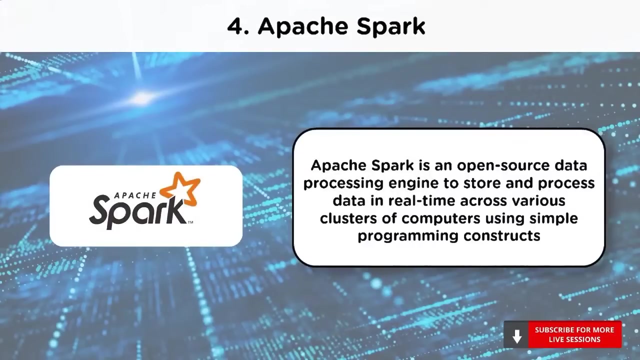 Again, to name a few, we have Amazon, Google and the American photo and video sharing social networking service, Instagram. That was all about R and Python. At number 4, we have Apache Spark. Apache Spark is an open-source engine developed specifically for handling large-scale data. 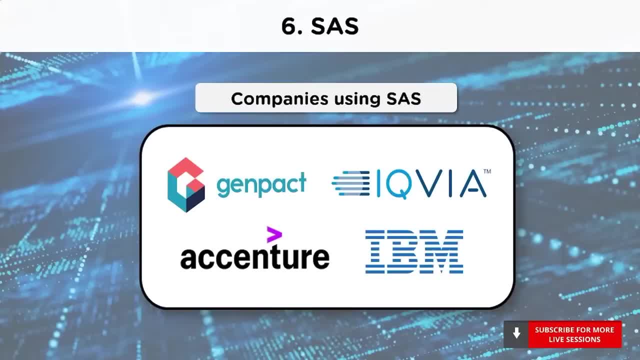 8 we have Talent. at number 7 we have Nine and at number 6 we have SaaS. So far. do you all agree with this list? Let us know in the comment section below. Let's now move on to the next 5 tools in our list. 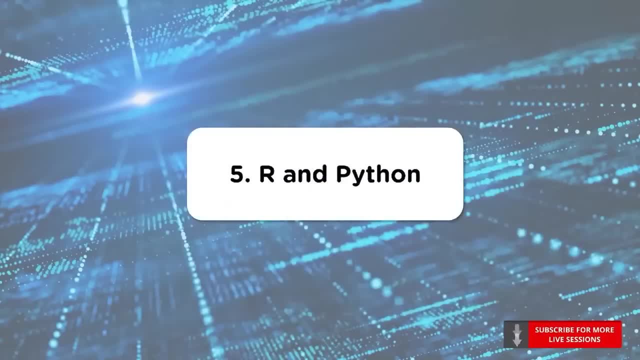 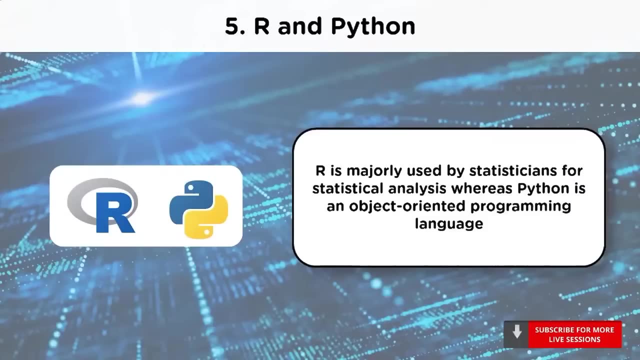 So at number 5 we have both R and Python. Yes, we have two of them in the 5th position. R is a programming language which is used for analysis as well. It has traditionally been used in academics and research. Python is a high-level programming language which has a Python data analysis library. 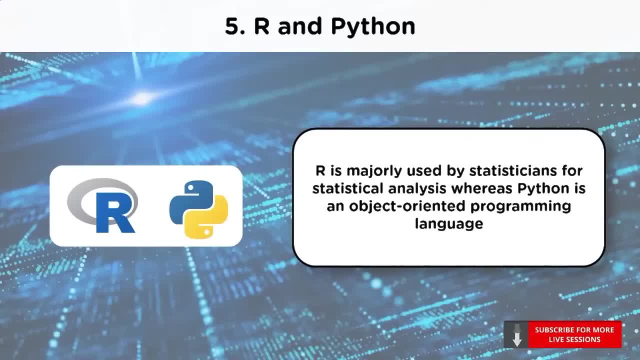 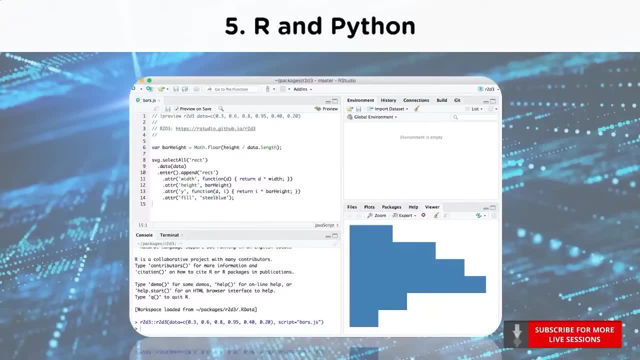 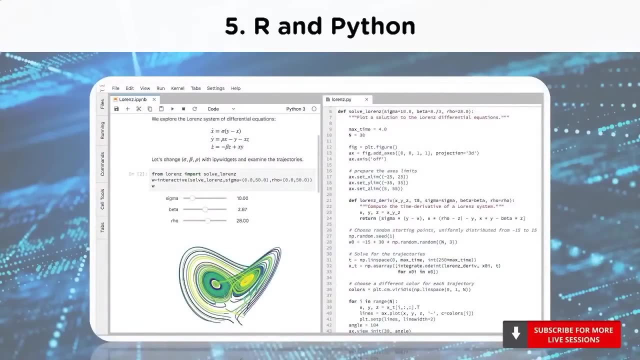 It is used for everything, Starting from importing data from Excel spreadsheets to processing them for analysis. This is the interface of R. Next up is the interface of the Python Jupyter Notebook. Let's now move on to the features of both R and Python. 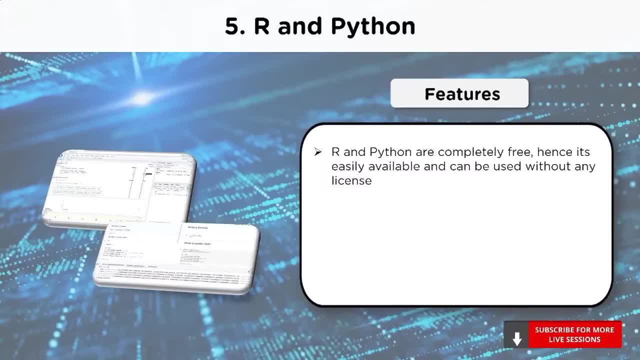 When it comes to the availability of R and Python, it is very easy. Both R and Python are completely free, Hence it can be used without any problems. So let's move on to the next 5 tools. R used to compute everything in memory, and hence the computations were limited. 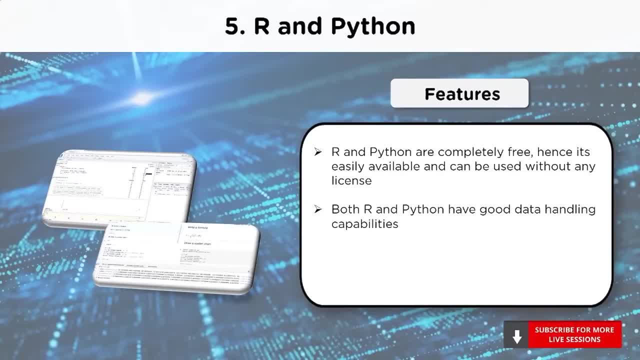 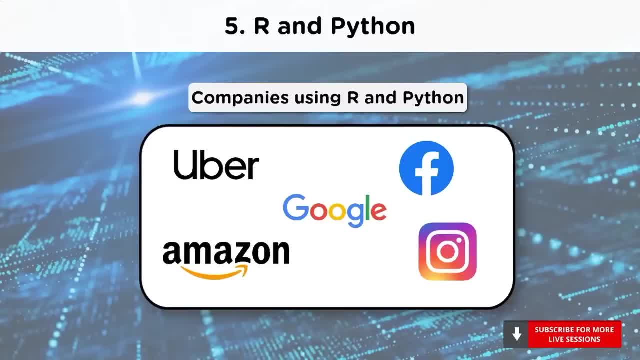 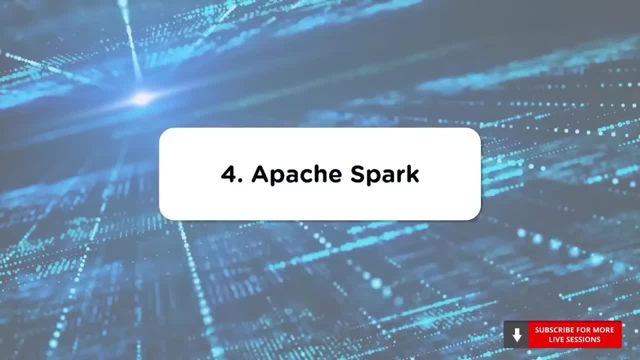 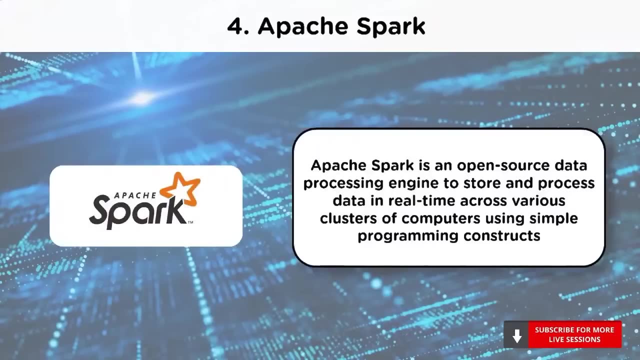 social networking service Instagram. That was all about R and Python. At number 4, we have Apache Spark. Apache Spark is an open-source engine developed specifically for handling large-scale data processing and analytics. Spark offers the ability to access data in a variety of sources, including Hadoop, Distributed. 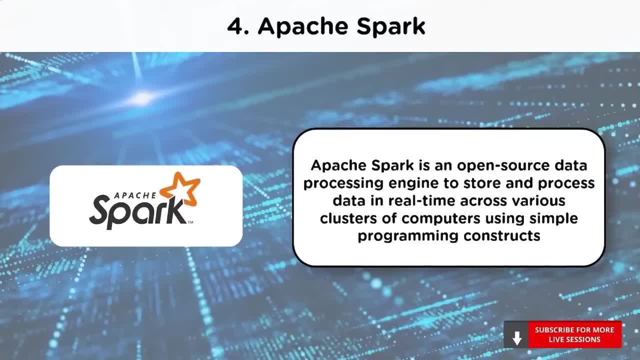 File System, OpenStack, Swift, Amazon S3, and Cassandra. It allows you to store and process data in real-time across various clusters of computers using simple programming constructs. Apache Spark is designed to accelerate analytics on Hadoop, while providing a complete suite of complementary tools that include a fully-featured machine learning library, a graph processing, 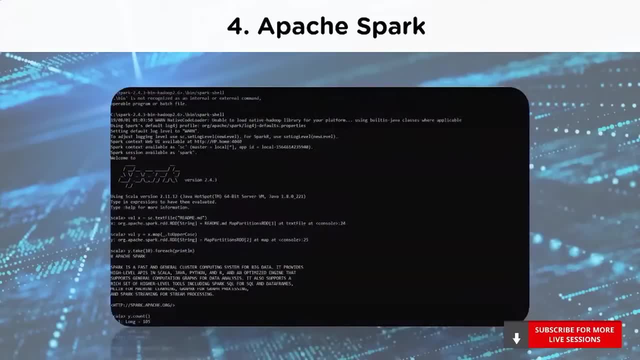 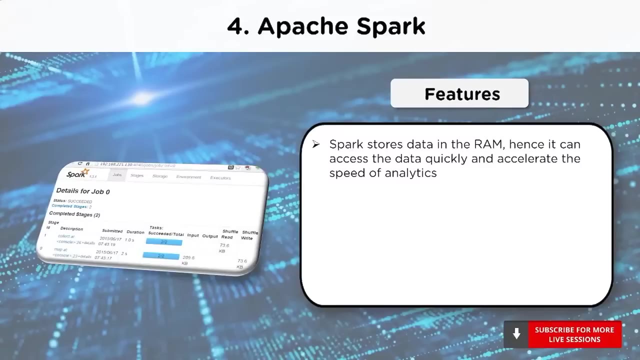 engine and stream processing. So this is how the interface of Apache Spark works. Now let's look at the important features of Apache Spark. Spark stores data in the RAM, Hence it can access the data quickly and accelerate the speed of analytics. Spark helps to run an application in a Hadoop. 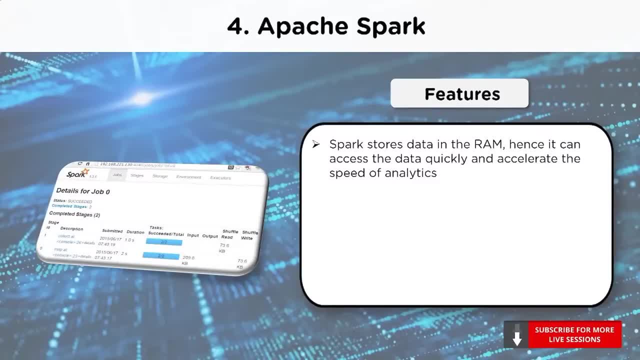 cluster up to 100 times faster in memory and 10 times faster when running on disk. It supports multiple languages and allows the developers to write applications in a Java, Scala, R or Python. Spark comes up with 80 high-level operators for interactive querying. 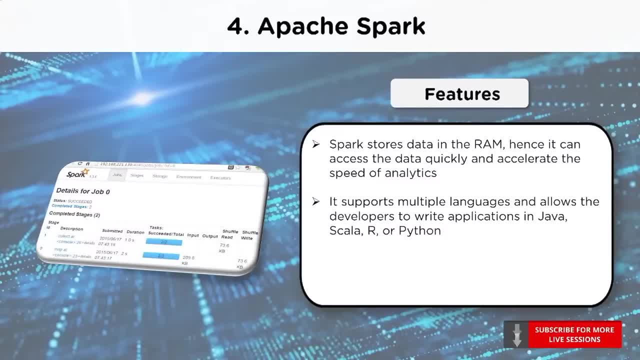 Spark code for batch processing, joint stream against historical data or run ad-hoc queries on stream. state Analytics can be performed better as Spark has a rich set of SQL queries, machine learning algorithms, complex analytics, etc. Apache Spark provides fault tolerance through Spark RDD. 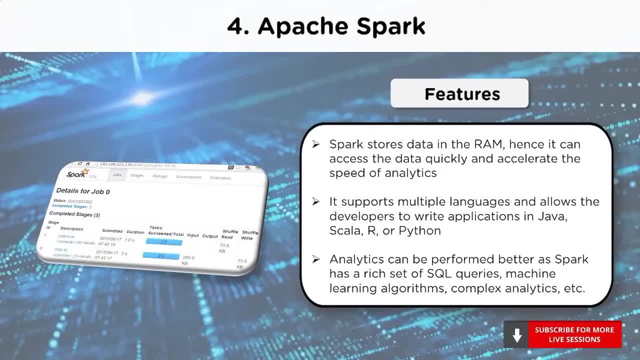 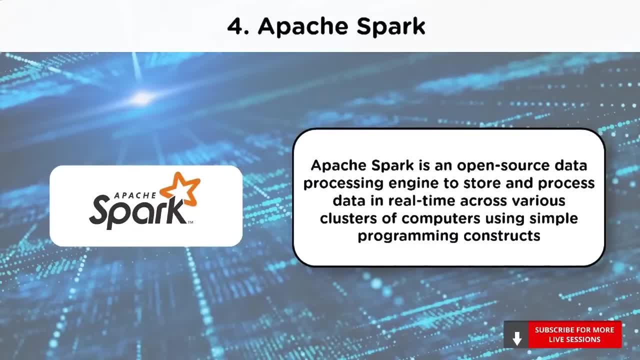 processing and analytics. Spark offers the ability to access data in a variety of sources, including Hadoop, Distributed File System, OpenStack, Swift, Amazon S3 and Cassandra. It allows you to store and process data in real-time Across various clusters of computers using simple programming constructs. 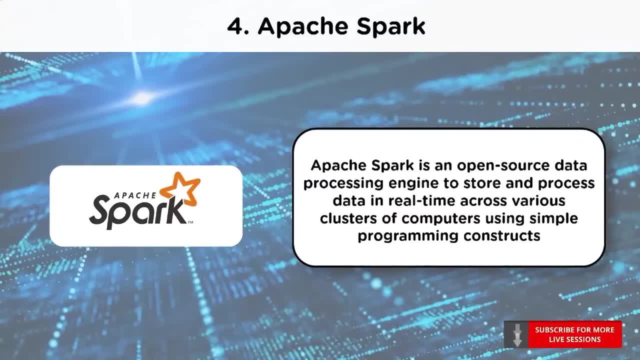 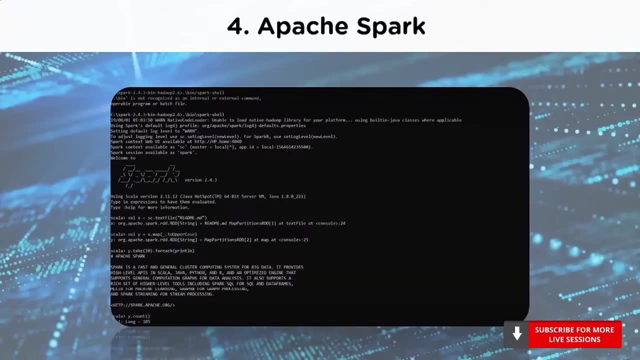 Apache Spark is designed to accelerate analytics on Hadoop while providing a complete suite of complementary tools that include a fully-featured machine learning library, a graph processing engine and stream processing. So this is how the interface of Apache Spark looks like. Now let's look at the important features of Apache Spark. 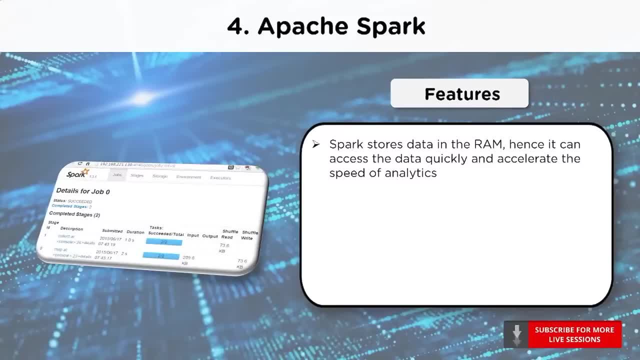 Spark stores data in the RAM, hence it can access the data quickly and accelerate the speed of analytics. Spark helps to run an application in a Hadoop cluster up to 100 times faster in memory and 10 times faster when running on disk. It supports multiple languages and allows the developers to write applications in Java. 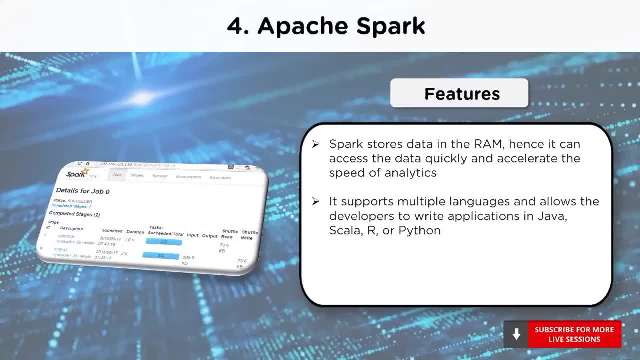 Scala R or Python. Spark comes up with 80 high-level operators for interactive querying. Spark code for batch processing, joint stream against historical data or run ad-hoc queries on stream. state Analytics can be performed better as Spark has a rich set of SQL queries. machine learning: 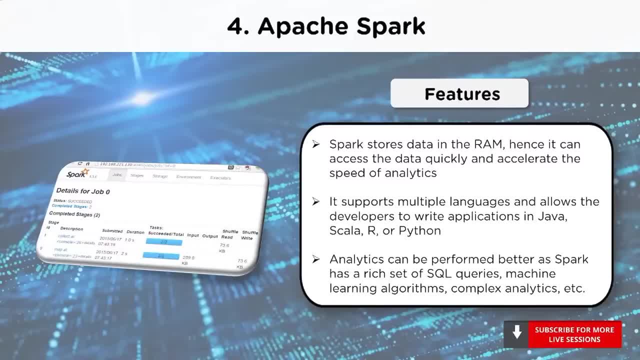 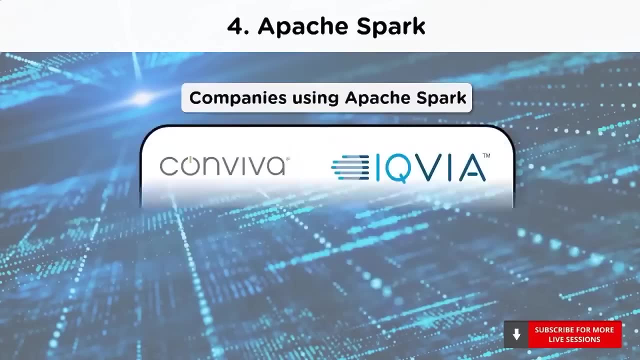 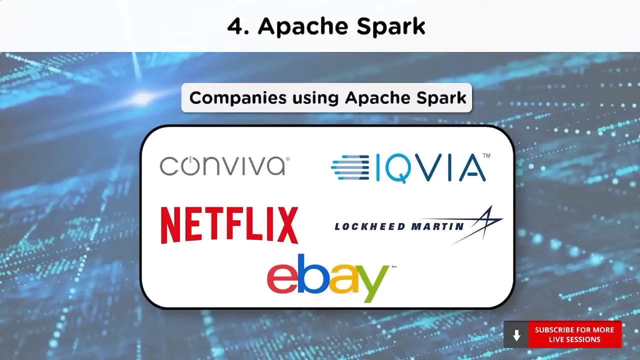 algorithms, complex analytics, etc. Apache Spark provides fault tolerance through Spark RDD. Spark Resilient Distributed Datasets are designed to handle the failure of any worker node in the cluster. Thus it ensures that the loss of data reduces to zero. Conviva, Netflix, IQVR, Lockheed Martin and eBay are some of the companies that use. 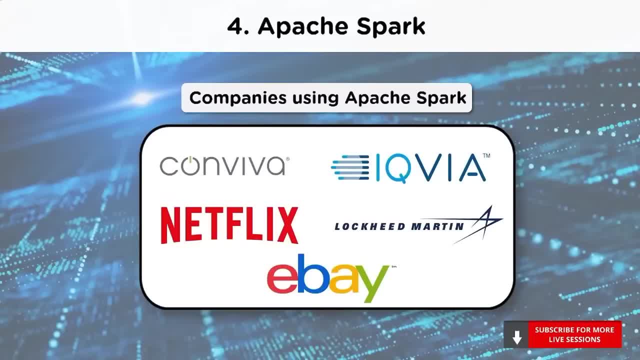 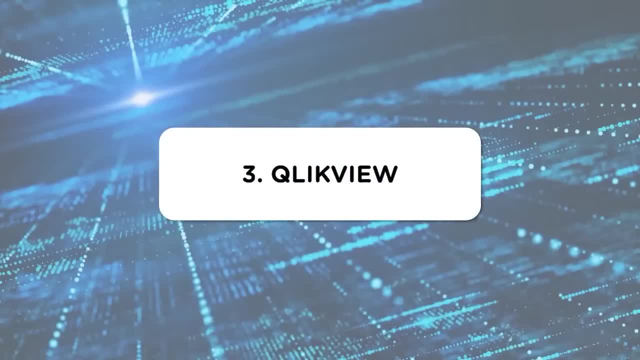 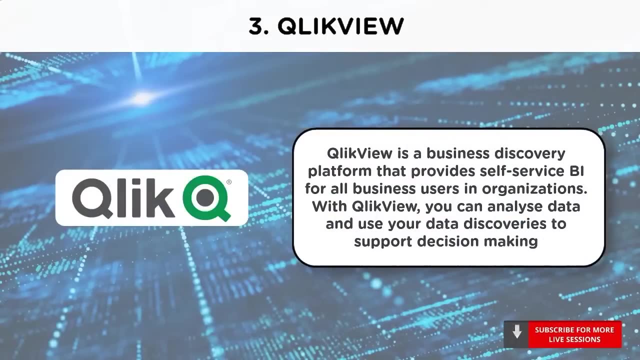 Apache Spark on a daily basis At number 3,. we have another important growing data analysis tool, ie Clickview. Clickview Software is a product of Qlik for business intelligence and data visualization. Clickview is a business discovery platform that provides self-service BI for all business. 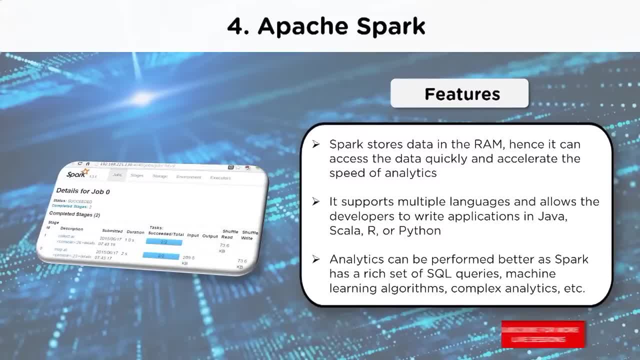 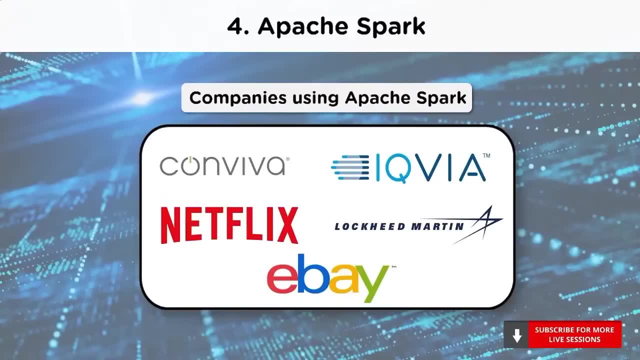 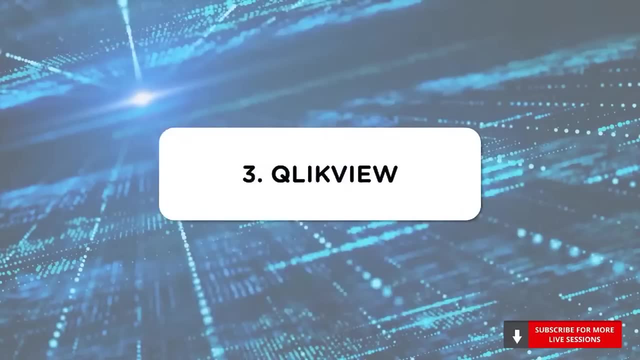 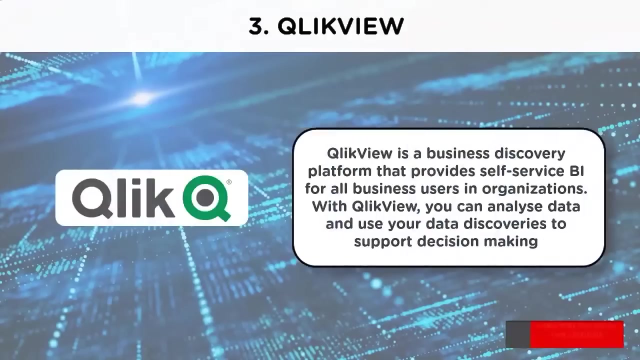 Spark RDD is a very powerful tool for data processing. американ RDD is the newest system and is the most advanced technology now in what some have called the α3D объяс jaar more over. Apple Posture. Clickview is a business discovery platform that provides self-service BI for all business users and organizations. 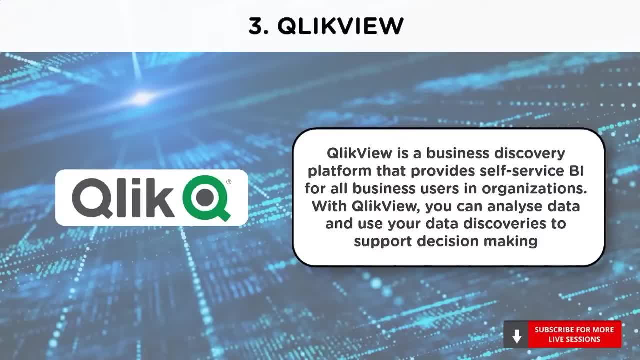 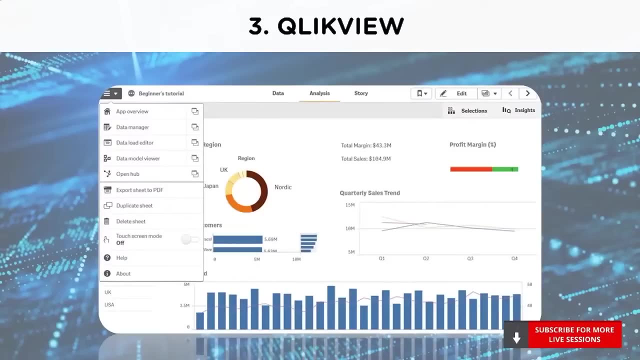 With Clickview, you can analyze data and use your data discoveries to support decision making. Clickview is a leading business intelligence and analytics platform. in Gartner Magic Quadrant On the screen, you can see how the interface of Clickview looks like. 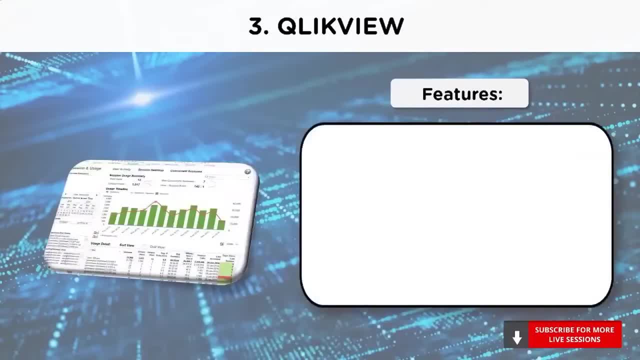 Now talking about its features. Clickview provides interactive guided analytics with in-memory storage technology. During the process of data discovery and interpretation of collected data, the Clickview software helps the user by suggesting possible interpretations. Clickview uses a new patent in-memory architecture for data storage. 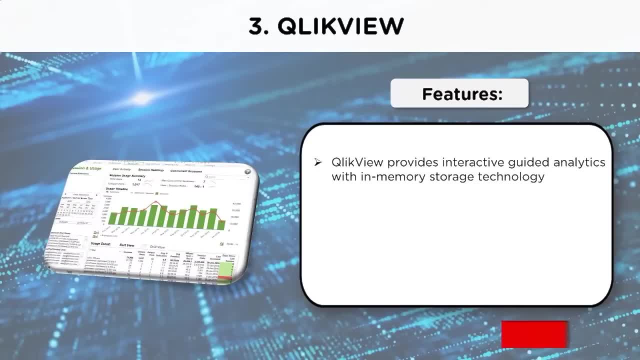 All the data from the different sources is loaded in the RAM of the system and it is ready to be retrieved from there. It has many features. It has the capability of efficient social and mobile data discovery. Social data discovery offers to share individual data insights within groups or out of it. 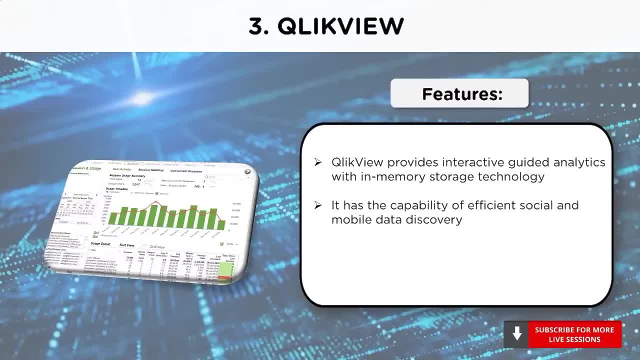 A user can add annotations as an addition to someone else's insights on a particular data report. Clickview supports mobile data discovery within an HTML5-enabled touch feature, which lets the user search the data and conduct data discovery interactively and explore other server-based applications. 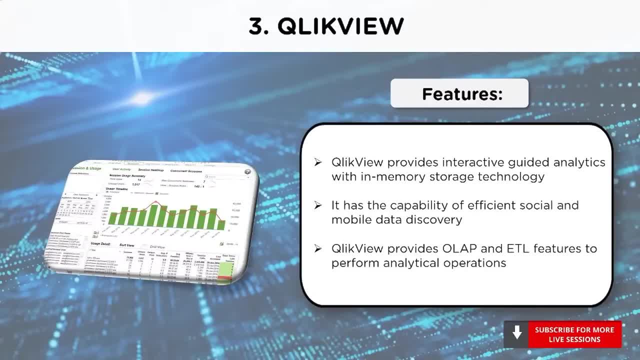 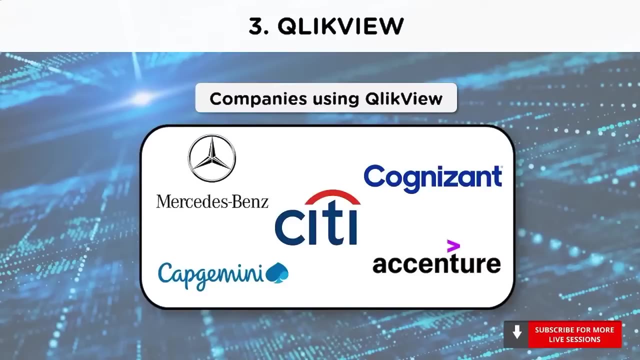 Clickview performs OLAP and ETL features to perform analytical operations, extract data from multiple sources, transform it for usage and load it to a data warehouse. The companies that can help you start your career in Clickview are Mercedes-Benz, Capgemini, Citibank, Cognizant and Accenture, to name a few. 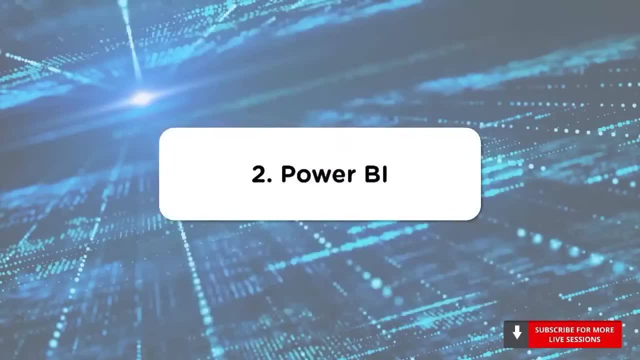 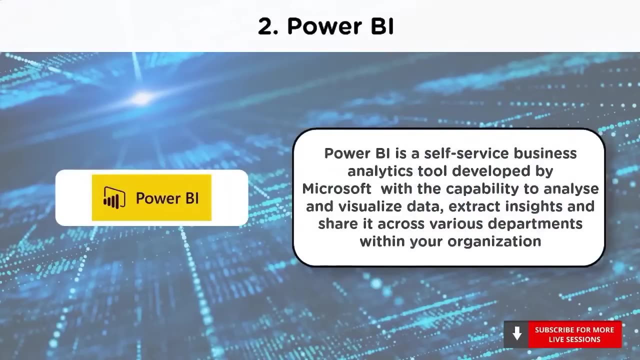 At number 2, we have Power BI. Power BI is the first mobile data security software developed by Google. It is the first mobile data security software to be developed by Google. Power BI is a business analytics solution that lets you visualize your data and share insights across your organization. 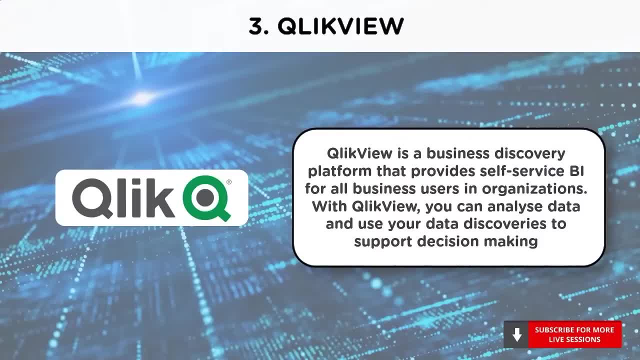 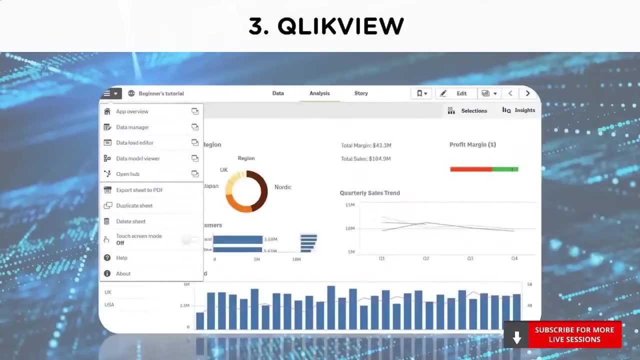 users and organizations. With Qlikview, you can analyze data and use your data discoveries to support decision making. Clickview is a leading business intelligence and analytics platform in Gartner Magic Quadrant. On the screen, you can see how the interface of Qlikview looks like. 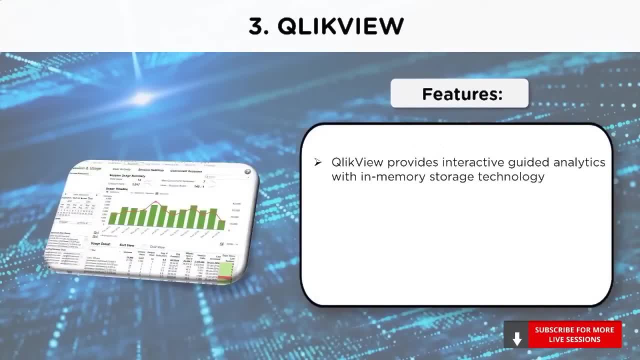 Now talking about its features. Qlikview provides interactive guided analytics with in-memory storage technology. During the process of data discovery and interpretation of collected data, the Qlikview software helps the user by suggesting possible interpretations. Qlikview uses a new patent in-memory architecture for data storage. 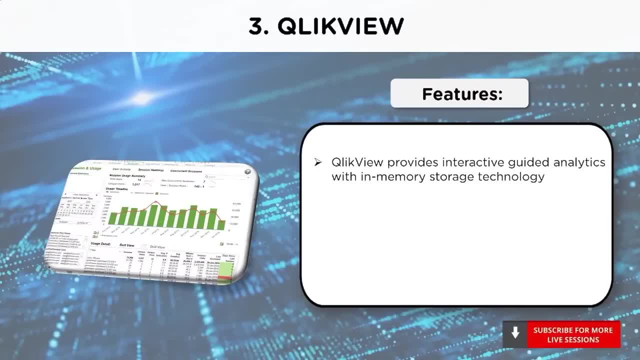 All the data from the different sources is loaded in the RAM of the system and it is ready to be retrieved from there. It has the capability of efficient social and mobile data discovery. Social data discovery offers to share individual data insights. Clickview has the capability of efficient social and mobile data discovery. 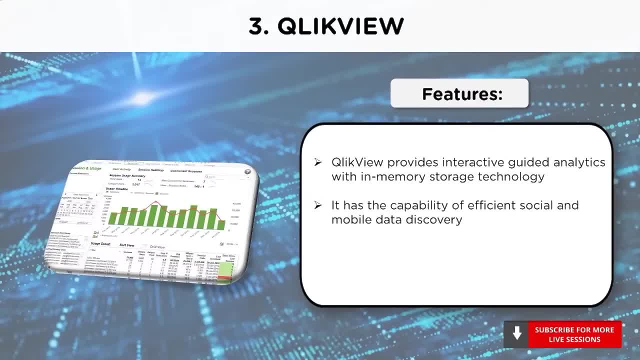 Social data discovery offers to share individual data insights. A user can add annotations as an addition to someone else's insights on a particular data report. Qlikview supports mobile data discovery within an HTML5-enabled touch feature which lets the user search the data and conduct data discovery interactively and explore other. 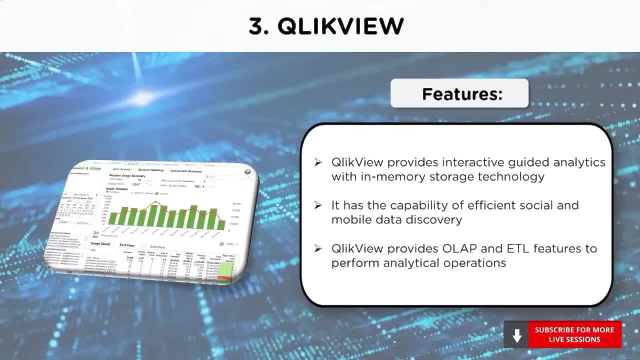 server-based applications. Qlikview performs OLAP and ETL features to perform analytical operations, extract data from multiple sources, transform its for-use data and other data. Qlikview is a leading business intelligence and analytics platform usage and load it to a data warehouse. 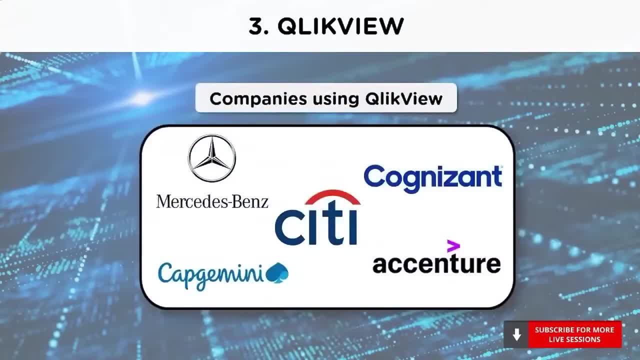 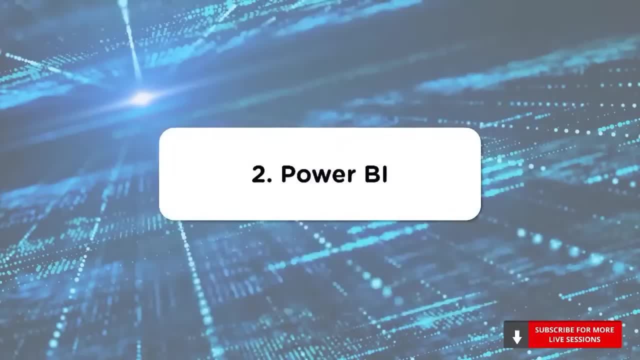 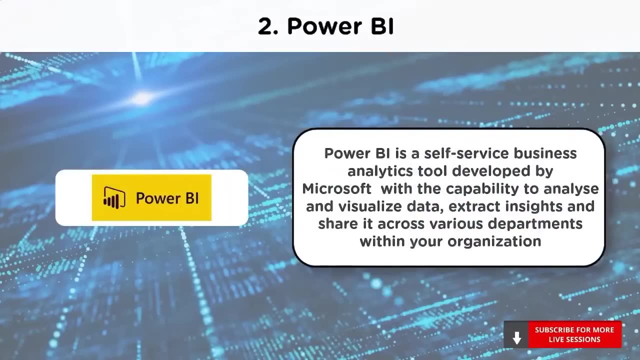 The companies that can help you start your career in ClickView are Mercedes-Benz, Capgemini, Citibank, Cognizant and Accenture, to name a few. At number 2, we have Power BI. Power BI is a business analytics solution that lets you visualize your data and share. 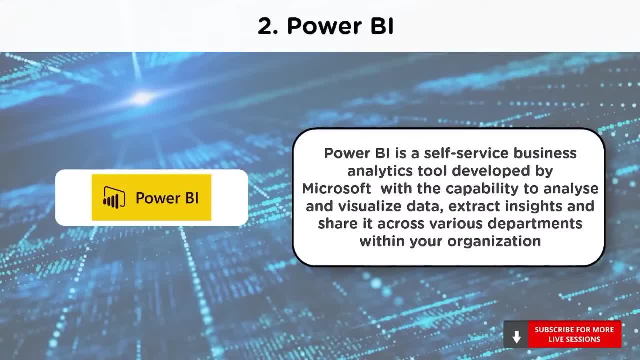 insights across your organization or embed them in your app or website. It can connect to hundreds of data sources and bring your data to life with live dashboards and reports. Power BI is the collective name for a combination of cloud-based apps and services that help. 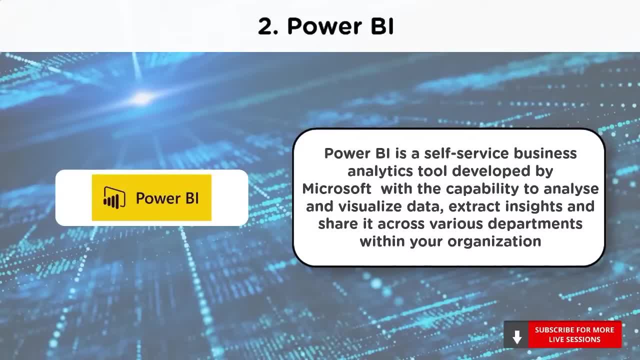 or embed them in your app or website. It can connect to hundreds of data sources and bring your data to life with live dashboards and reports. Power BI is the collective name for a combination of cloud-based apps and services that help organizations collate, manage and analyze data from a variety of sources. 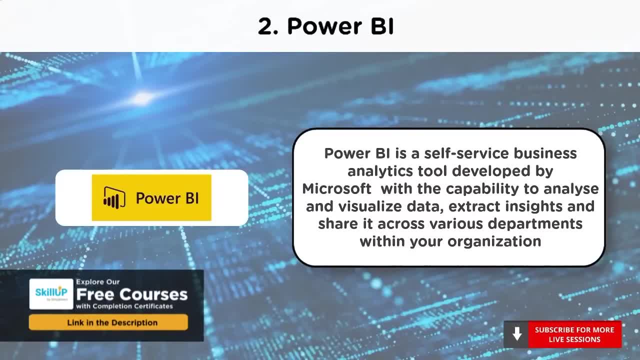 through a user-friendly interface. Power BI is built on the foundation of Microsoft Excel and has several components, such as Windows desktop application, called Power BI Desktop, and online software as a service, called Power BI Service. mobile Power BI apps available on Windows phones and tablets, as well as for iOS and Android devices. 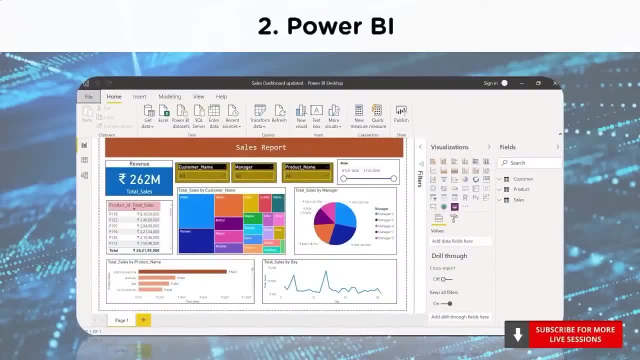 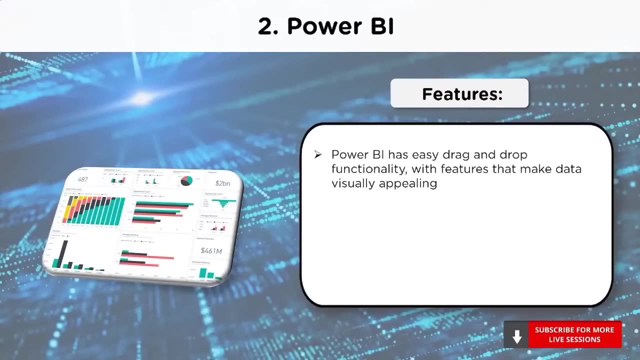 Here is how the Power BI interface looks like. As you can see, there is a visually interactive sales report with different charts and graphs. Moving on to the features of Power BI, It has an easy drag and drop functionality with features that make data visually appealing. 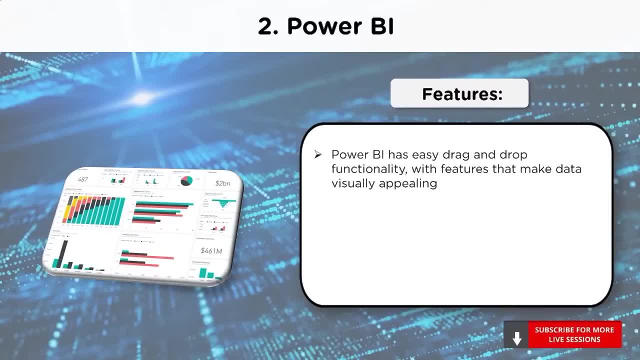 You can create reports without having the knowledge of any programming language. Power BI helps users see not only what's happened in the past and what's happening in the present, but also what might happen in the future. It offers a wide range of detailed and attractive visualizations to create reports and dashboards. 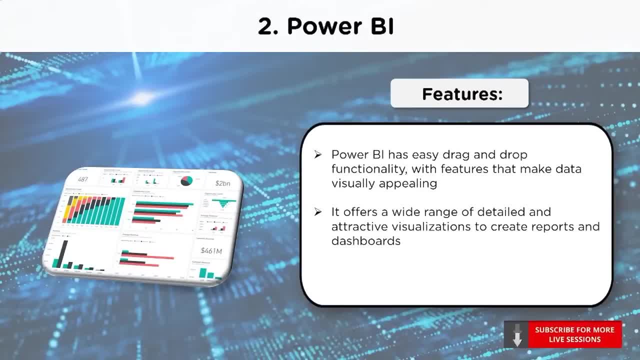 You can select several charts and graphs from the visualization pane. Power BI has machine learning capabilities with which it can spot patterns in data and use those patterns to make informed predictions and run what-if scenarios. Power BI supports multiple data sources, such as Excel, TechCSV, Oracle, C++, Excel. 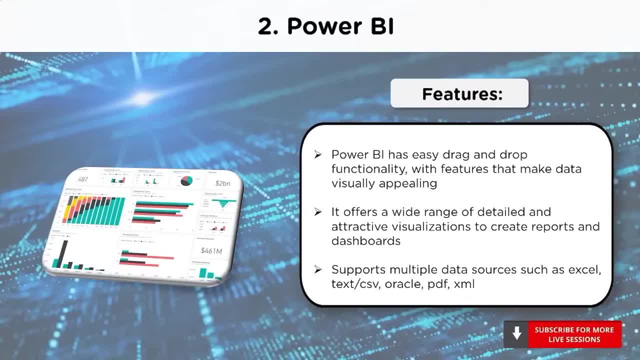 SQL Server PDF and XML files. The platform integrates with other popular business management tools like SharePoint, Office 365, and Dynamics 365, as well as other non-Microsoft products like Spark, Hadoop, Google Analytics, SAP, Salesforce and MailChimp. 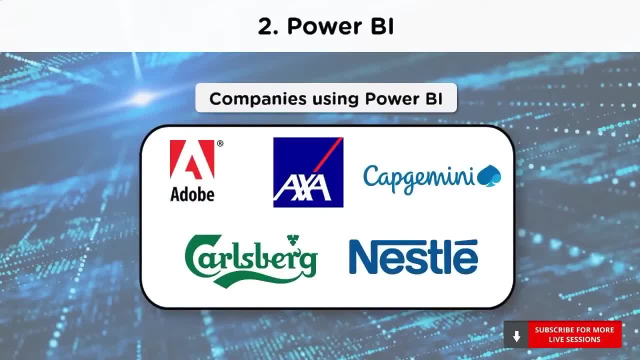 Some of the companies using Power BI are Adobe, AXA, Carlsberg, Capgemini and Nestle, Moving on to the next tool. So any guesses as to what we have at number one You can comment in the chat section below. 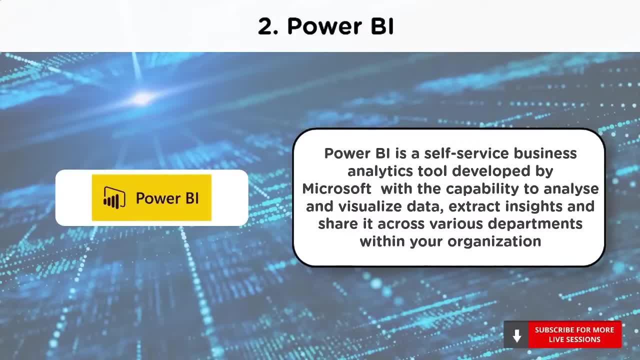 organizations collate, manage and analyze data from a variety of sources through a user-friendly interface. Power BI is built on the foundation of Microsoft Edge Excel and has several components, such as Windows desktop application, called Power BI Desktop, and online software as a service, called Power BI Service. mobile Power BI apps available. 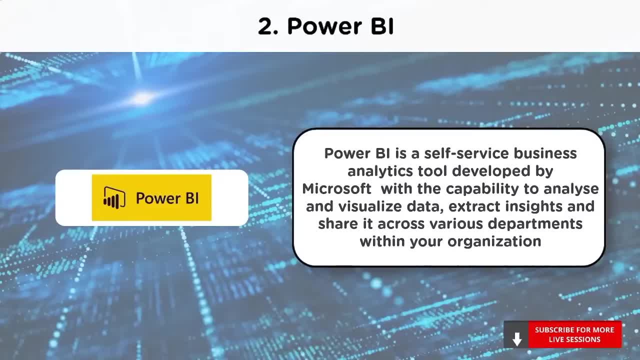 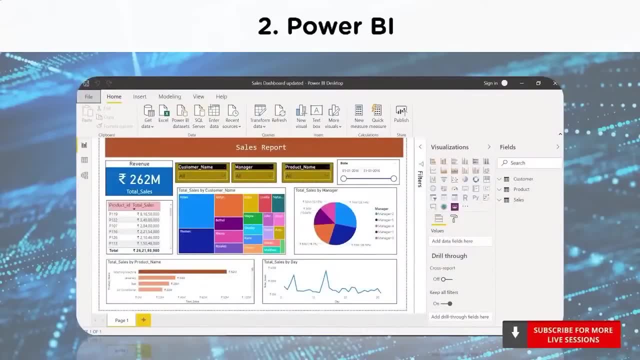 on Windows phones and tablets, as well as for iOS and Android devices. Here is how the Power BI interface looks like. As you can see, there is a visually interactive sales report with different charts and graphs. Moving on to the features of Power BI, 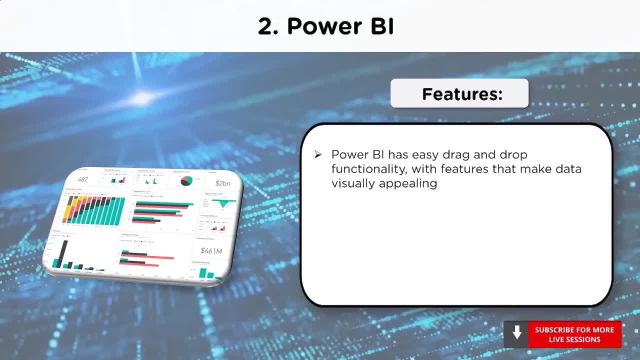 It has an easy drag-and-drop functionality. with features that make data visually appealing, You can create reports without having the knowledge of any programming language. Power BI helps users see not only what's happened in the past and what's happening in the present. 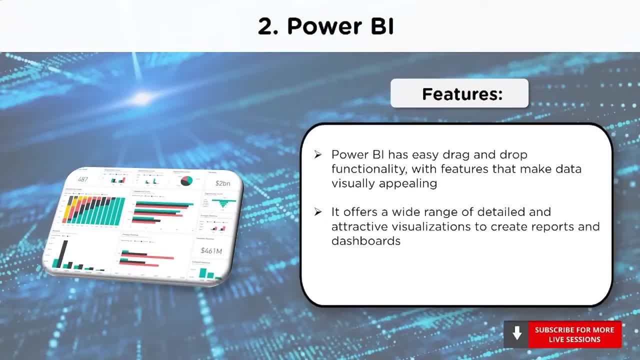 but also what might happen in the future. It offers a wide range of detailed and attractive visualizations to create reports and dashboards. You can select from a wide range of detailed and attractive visualizations to create reports and dashboards. You can select several charts and graphs from the visualization pane. 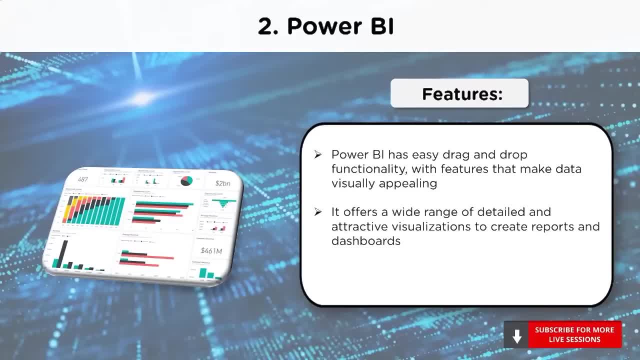 Power BI has machine learning capabilities with which it can spot patterns in data and use those patterns to make informed predictions and run what-if scenarios. Power BI supports multiple data sources, such as Excel, TechCSV, Oracle, SQL Server, PDF and XML files. 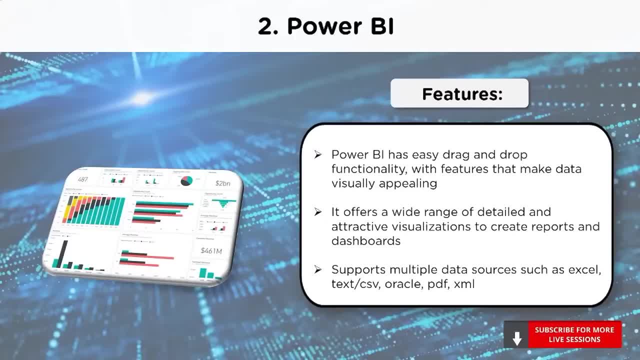 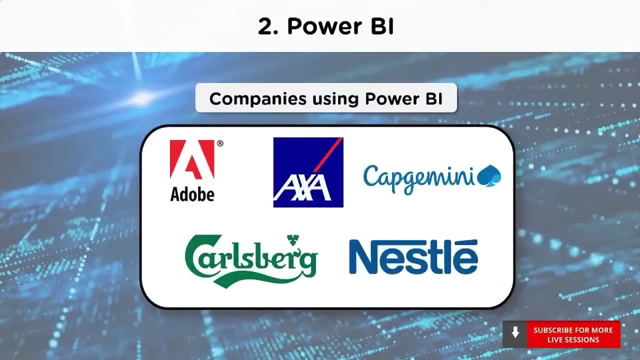 The platform integrates with other popular business management tools like SharePoint, Office 365, and Dynamics 365., As well as other non-Microsoft products like Spark, Hadoop, Google Analytics, SAP, Salesforce and MailChimp. Some of the companies using Power BI are Adobe, AXA, Carlsberg, Capgemini and Nestle. 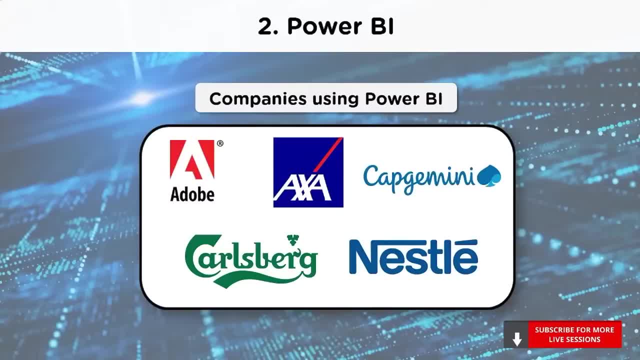 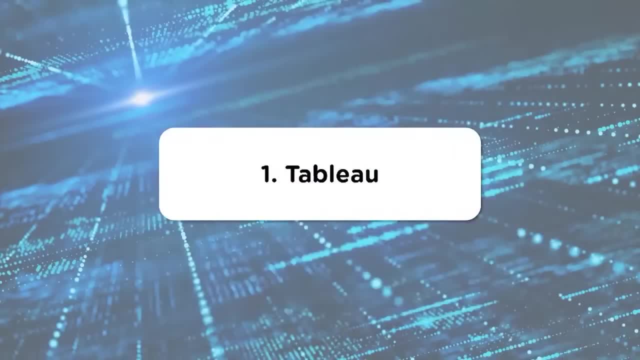 Moving on to the next tool. So any guesses as to what we have at number 1?? You can comment in the chat section below. Finally, we have the next tool. Finally, on the top of the pyramid, we have Tableau. 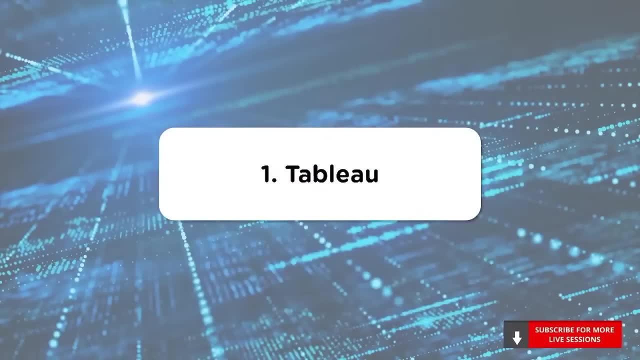 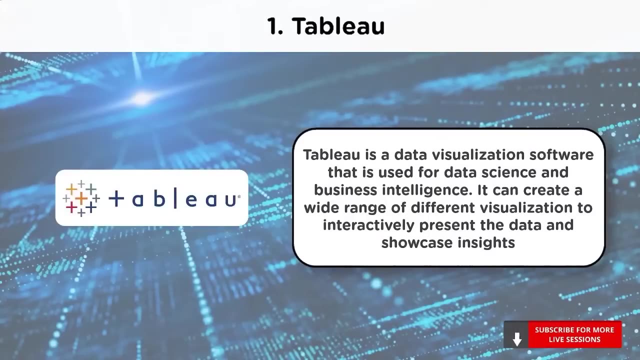 Finally, on the top of the pyramid, we have Tableau. Gartner's Magic Quadrant of 2020 classified Tableau as a leader in business intelligence and data analysis. Tableau Interactive Data Visualization Software Company was founded in Jan 2003 in Mountain View, California. 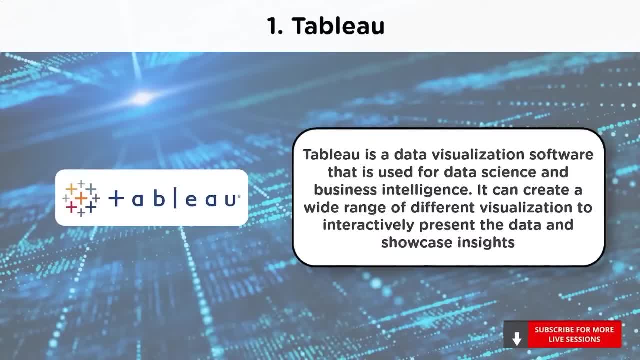 Tableau is a data visualization software that is used for data science and business intelligence. It can create a wide range of different visualization to interactively present the data and showcase insights. The important products of Tableau are: Tableau Desktop, Tableau Public, Tableau Server, Tableau Online and Tableau Reader. 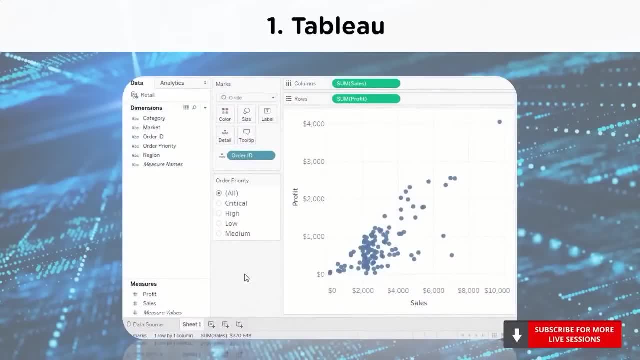 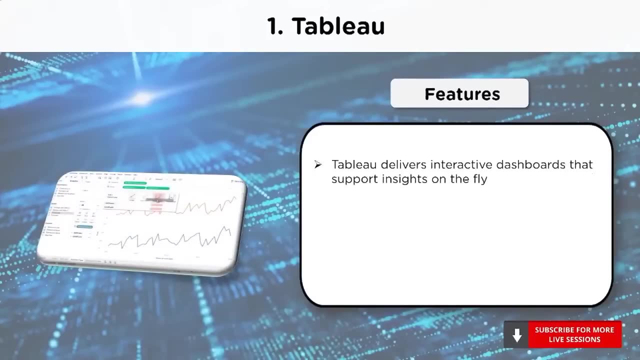 This is how the interface of Tableau Desktop looks like. Now coming to the features of Tableau. Data analysis is very fast with Tableau and the visualizations created are in the form of dashboards and worksheets. Tableau delivers interactive dashboards that support insights on the fly. 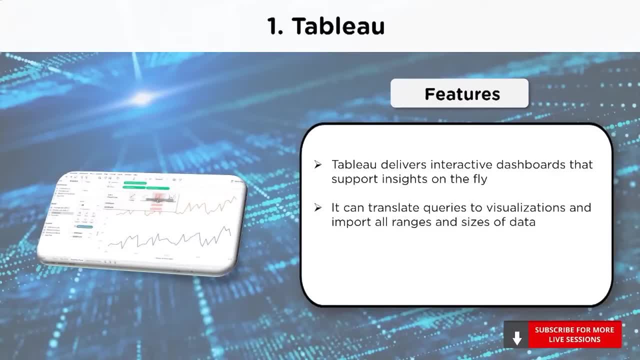 It can translate queries to visualizations and import all ranges and sizes of data. Writing simple SQL queries can help join multiple datasets and then build reports out of it. You can create transparent filters, parameters and highlights. Tableau allows you to ask questions, spot trends and identify opportunities. 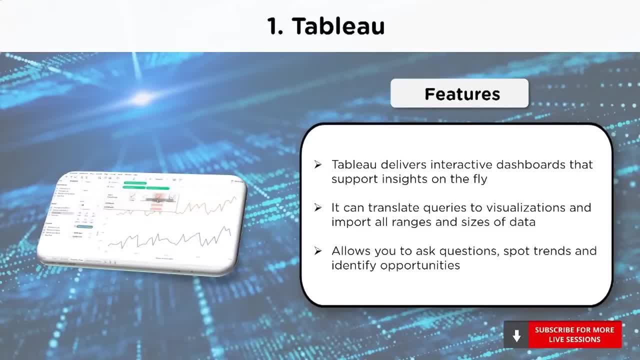 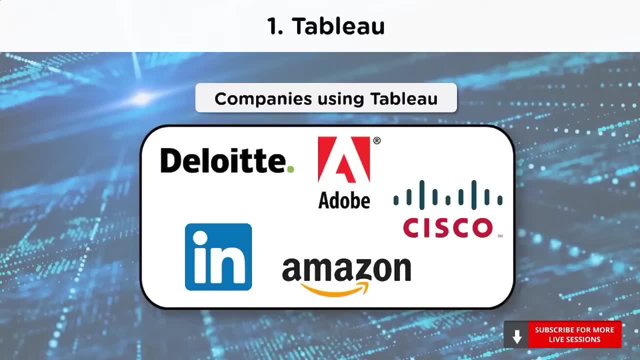 With the help of Tableau Online, you can connect with cloud databases, Amazon, Redshift and Google BigQuery. The companies using Tableau are Deloitte, Adobe, Cisco, LinkedIn and the American e-commerce giant Amazon, to name a few. 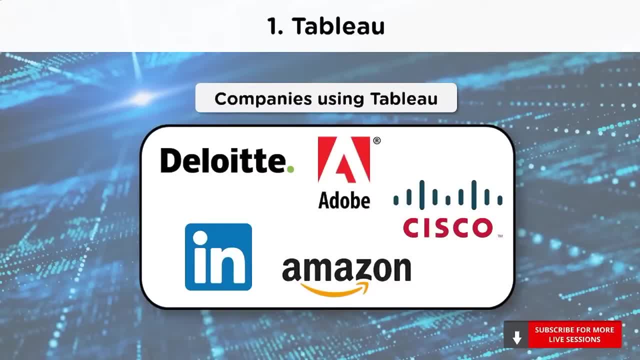 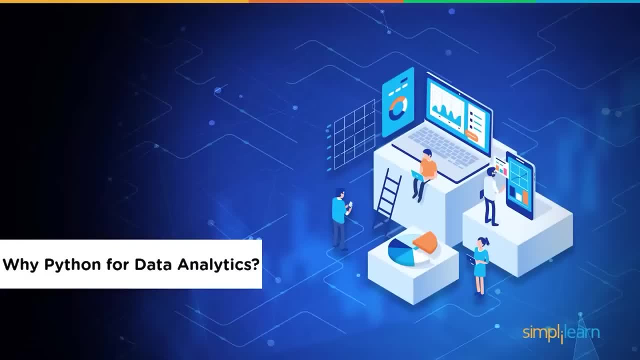 And there you go. Those are the top 10 data analysis tools. Since this is data analysis, we are going to talk a little bit about Tableau. Since this is data analysis with Python, we have to ask the question: why Python for data analytics? 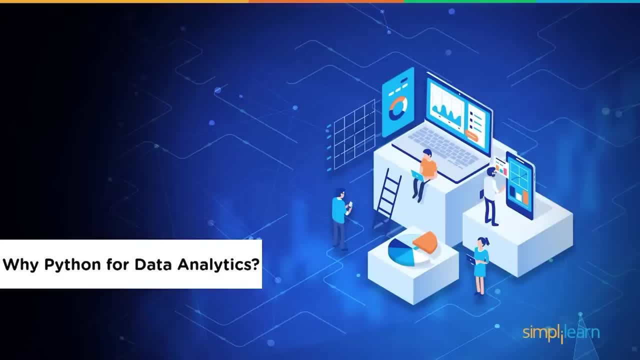 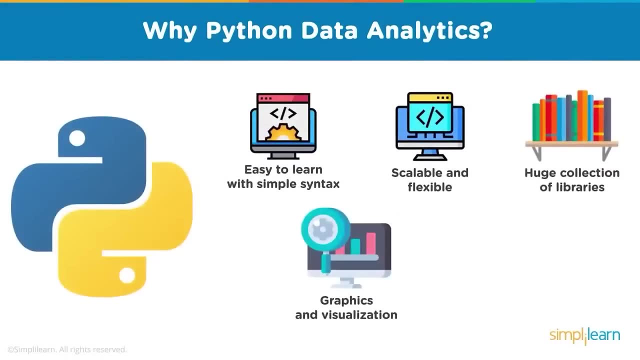 I mean there's C++, there's Java, there's NET from Microsoft. Why do people go to Python for it? So a number of reasons. One: it's easy to learn with simple syntax. You don't have a very high typeset like you do in Java and other coding. 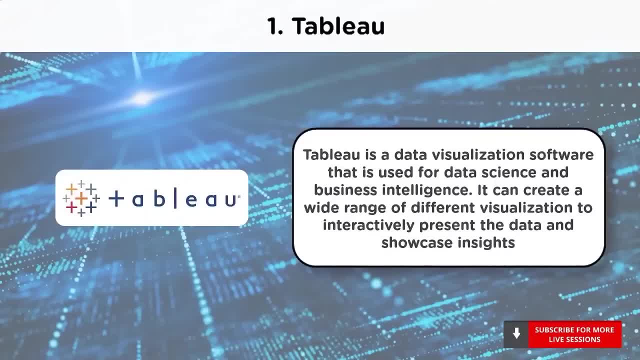 Gartner's Magic Quadrant of 2020 classified Tableau as a leader in business intelligence and data analysis. Tableau Interactive Data Visualization Software Company was founded in Jan 2003 in Mountainview, California. Tableau is a data visualization software that is used for data science and business intelligence. 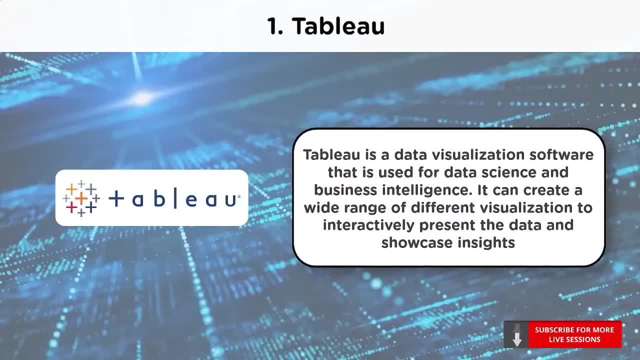 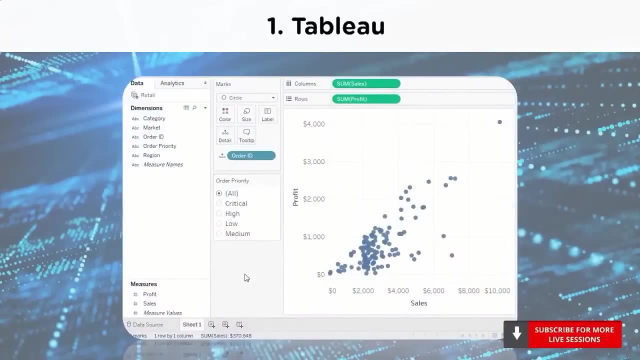 It can create a wide range of different visualization to interactively present the data and show case insights. The important products of Tableau are Tableau Desktop, Tableau Public, Tableau Server, Tableau Online and Tableau Reader. This is how the interface of Tableau Desktop looks like. 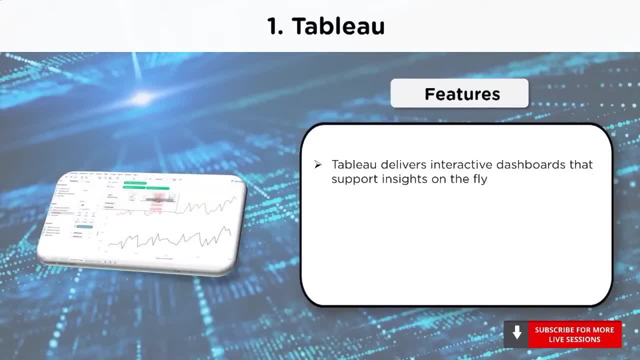 Now coming to the features of Tableau. Data analysis is very fast with Tableau and the visualizations created are in the form of dashboards and worksheets. Tableau delivers interactive dashboards that support the data analysis process. Tableau supports insights on the fly. 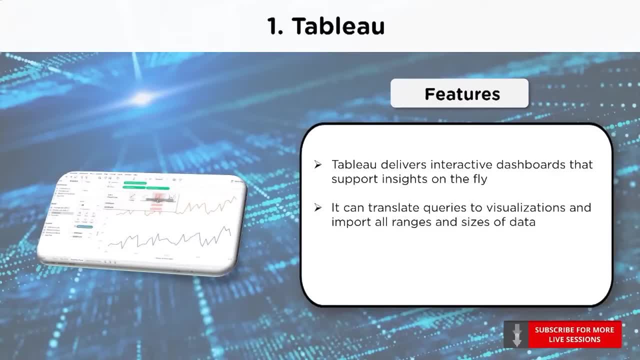 It can translate queries to visualizations and import all ranges and sizes of data. Writing simple SQL queries can help join multiple data sets and then build reports out of it. You can create transparent filters, parameters and highlighters. Tableau allows you to ask questions, spot trends and identify opportunities. 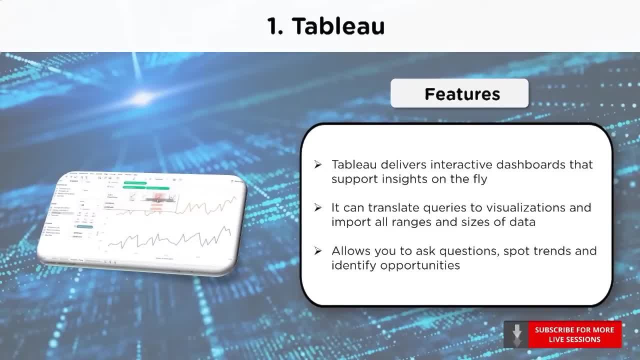 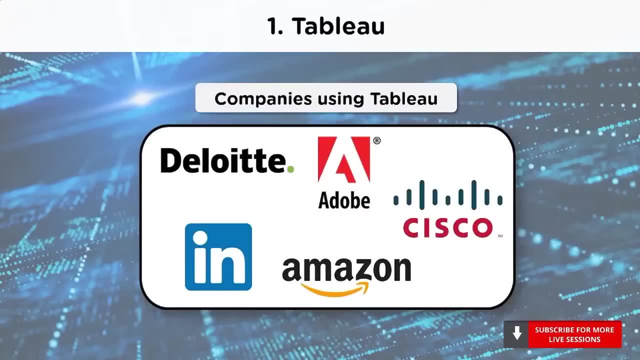 With the help of Tableau Online, you can connect with cloud databases, analytics and data analysis tools. You can also use Tableau Online Amazon Redshift and Google BigQuery. The companies using Tableau are Deloitte, Adobe, Cisco, LinkedIn and the American e-commerce. 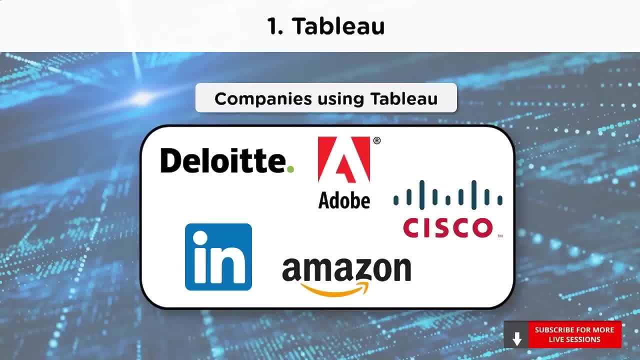 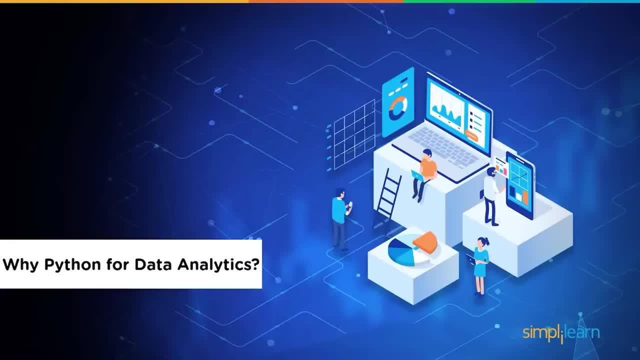 giant Amazon, to name a few. And there you go. Those are the top 10 data analysis tools. Since this is data analysis with Python, we've got to ask the question: why Python for data analytics? I mean, there's C++, there's Java, there's NET from Microsoft. 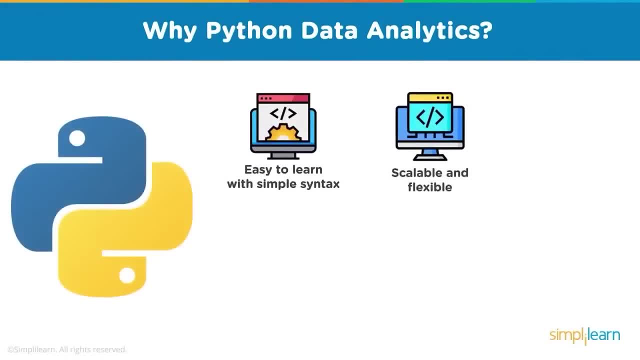 Why, Well, go to Python for it? So a number of reasons. One: it's easy to learn with simple syntax. You don't have a very high type set like you do in Java and other coding, so it allows you to kind of be a little lazy in your programming. 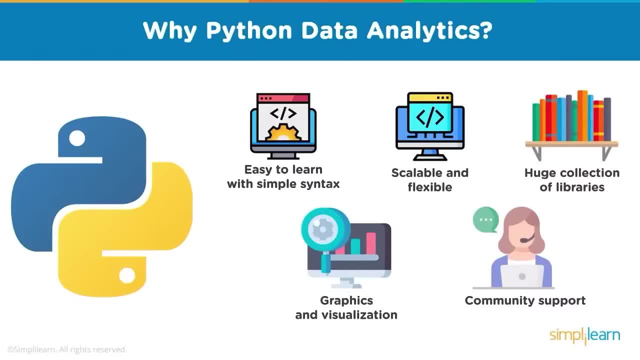 So it allows you to kind of be a little lazy in your programming. That doesn't mean that it can't be set that way and that you don't have to be careful. It just means you can spin up a code much quicker in Python. 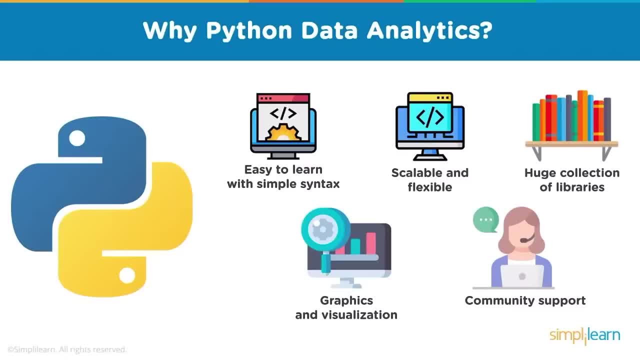 The same amount of code to do something in Python, a lot of times is one, two or three or four lines, Where, when I did the same thing, say, in Java, I found myself with 10,, 12,, 13,, 20 lines, depending on what it was. 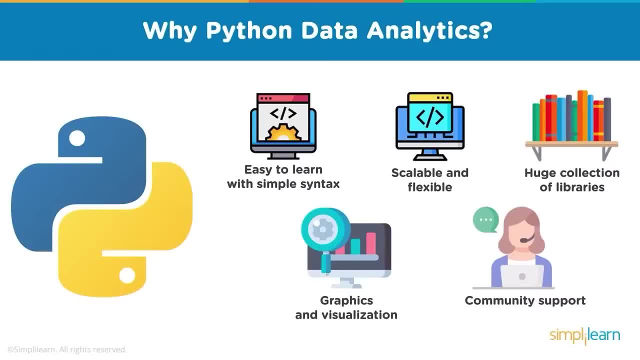 It's very scalable and flexible. So there's our flexibility, because you can do a lot with it And you can easily scale it up. You can go from something on your machine to using PySpark into the Spark environment and spread that across hundreds, if not thousands, of servers. 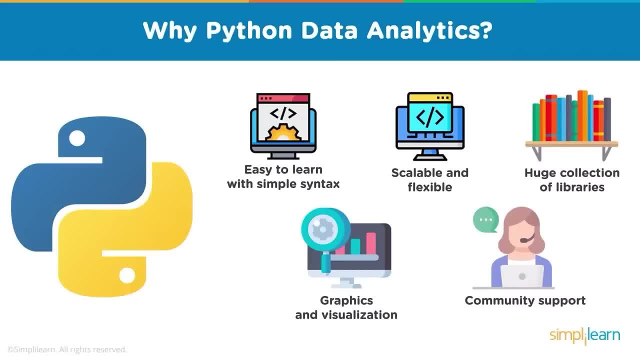 across terabytes of data or petabytes of data, So it's very scalable. There's a huge collection of libraries. This one's always interesting because Java has a huge collection of libraries. C has a huge collection of libraries. NET does. 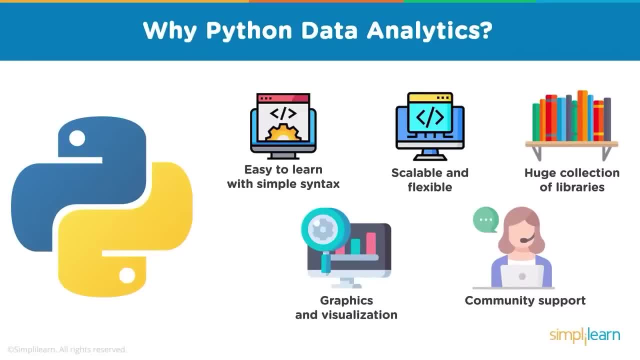 And they're always in competition to get those libraries out. Scala for your Spark- All those have huge collections of libraries. This is always changing But because Python's open source, you almost always have easy-to-access libraries that anybody can use. You don't have to go check your licensing and have special licensing like you do in some packages. 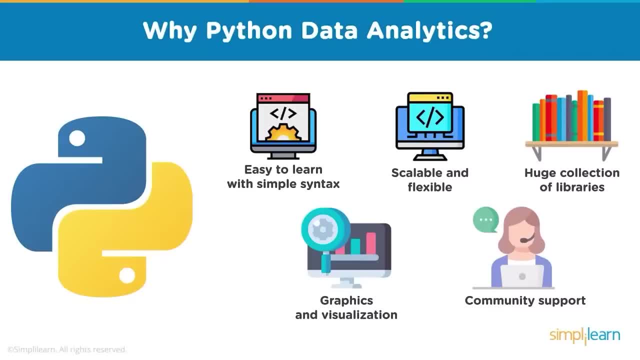 Graphics and visualization. They have a really powerful package for that, So it makes it easy to create nice displays for people to read. And community support. Because Python is open source, it has a huge community that supports it. You can do a quick Google and probably find a solution for almost anything you're working on. 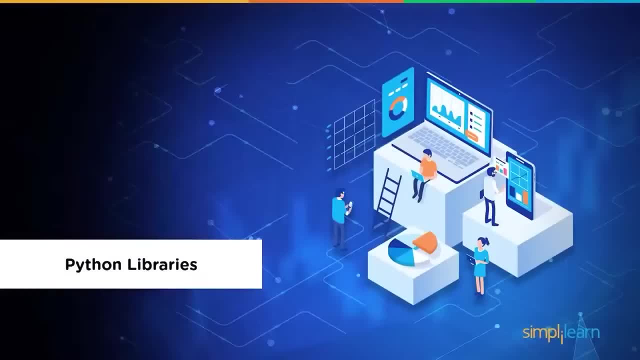 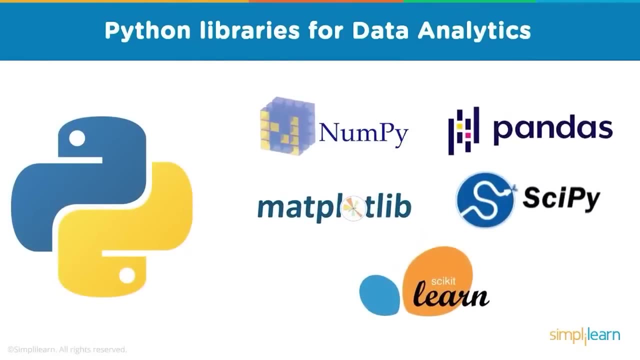 Python libraries. Let's bring it together: We have data analytics and we have Python. So when we're talking data analytics, we're talking Python libraries for data analytics, And the big five players are NumPy, Pandas, Matplot Library, SciPy, which is going to be in the background. 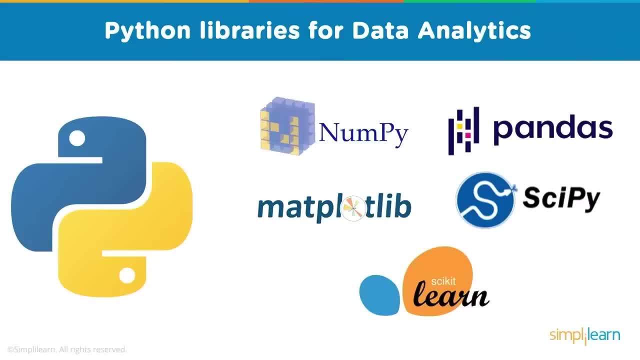 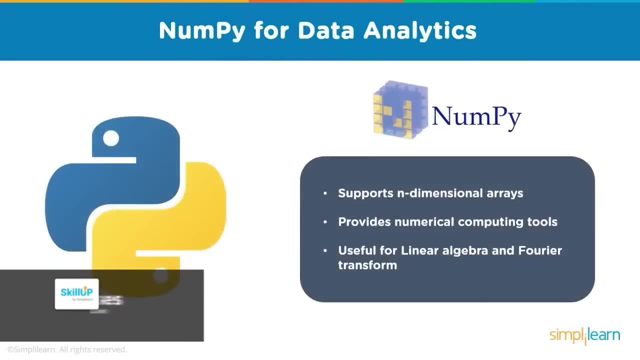 So we're not going to talk too much about the scientific formulas in SciPy And Scikit. So NumPy supports n-dimensional arrays, Provides numerical computing tools Useful for linear algebra and Fourier transform, And you can think of this as just a grid of numbers. 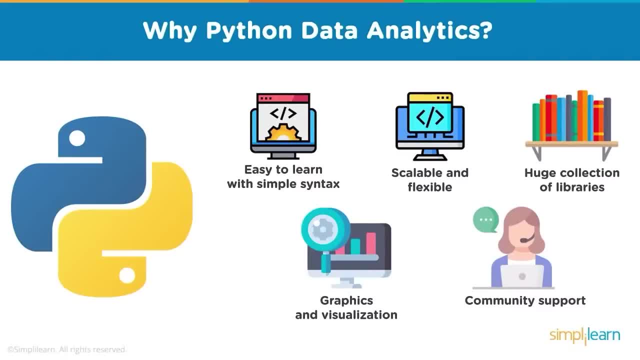 That doesn't mean that it can't be set that way and that you don't have to be careful. It just means you can spin up a code much quicker in Python. The same amount of code to do something in Python a lot of times is one, two or three. 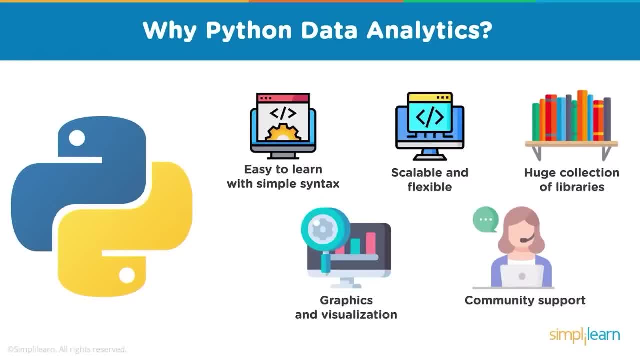 or four lines, Where, when I did the same thing, say in Java, I found myself with 10,, 12,, 13,, 20 lines, depending on what it was. It's very scalable and flexible. So there's our flexibility, because you can do a lot with it and you can easily scale. 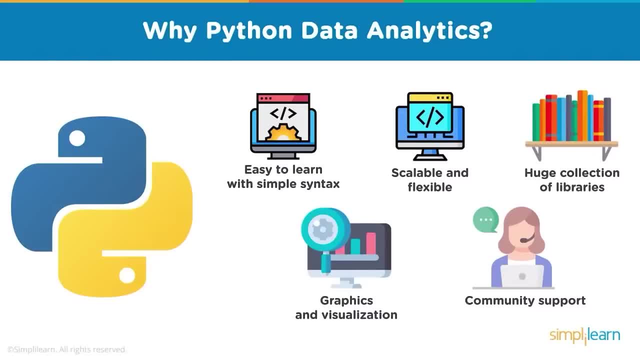 it up. You can go from something on your machine to using PySpark into the Spark environment and spread that across hundreds, if not thousands, of servers, across terabytes of data or petabytes of data, So it's very scalable. There's a huge collection of libraries. 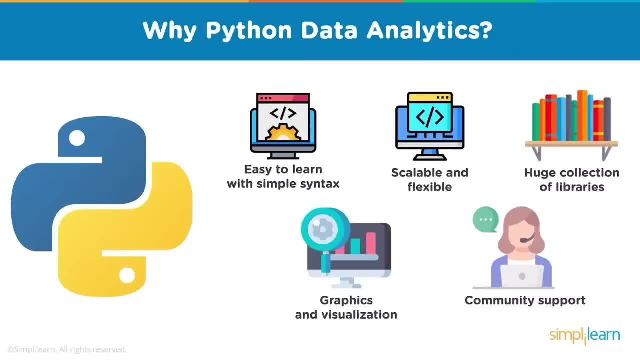 This one's always interesting because Java has a huge collection of libraries. C has a huge collection of libraries, NET does, and they're always in competition to get those libraries out. Scala for your Spark- All those have huge collections of libraries. 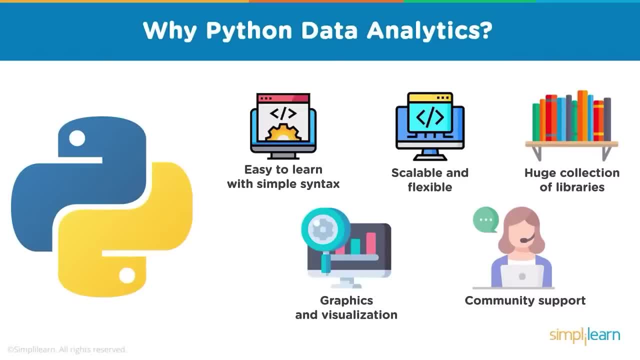 This is always changing, but because Python's open source, you almost always have easy-to-access libraries that anybody can use. You don't have to go check your licensing and have special licensing like you do in some packages- Graphics and visualization- They have a really powerful package for that, so it makes it easy to create nice displays. 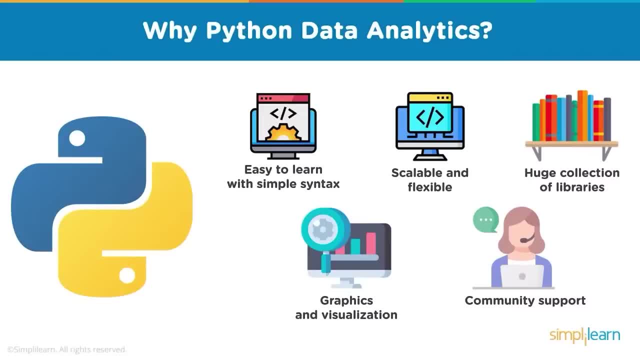 for people to read And community support. Because Python is open source, it has a huge community that supports it. You can do a quick Google and probably find a solution for almost anything. you're working on Python libraries. Let's bring it together. 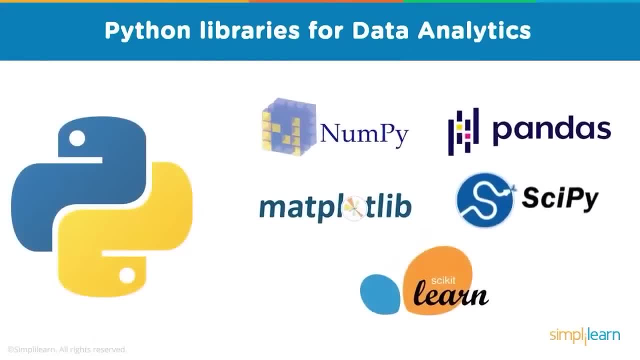 We have data analytics and we have Python. So when we're talking data analytics, we're talking Python libraries for data analytics, And the big five players are NumPy, Pandas, MatplotLibrary, SciPy, which is going to be in the background, so we're not going 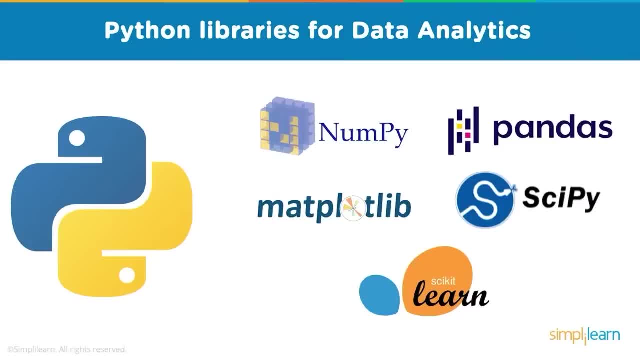 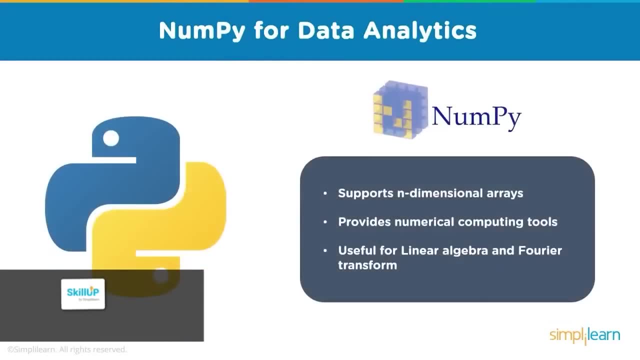 to talk too much about the scientific formulas in SciPy and Scikit. So NumPy supports n-dimensional arrays, provides numerical computing tools useful for linear algebra and Fourier transform, And you can think of this as just a grid of numbers and you can even have a grid inside. 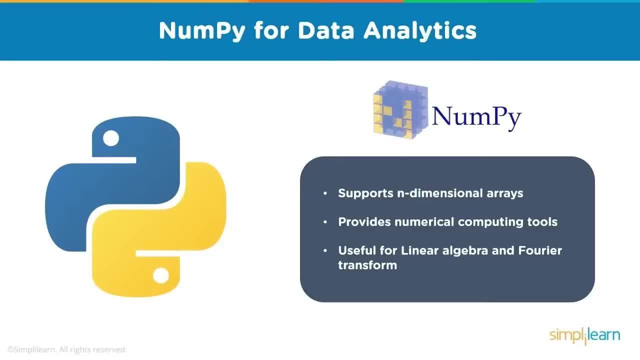 And you can even have a grid inside a grid, Or data. It's not even numbers, because you can also put words and characters and just about anything into that array, But you can think of a grid and then you can have a grid inside a grid and you end up with a nice three-dimensional array. 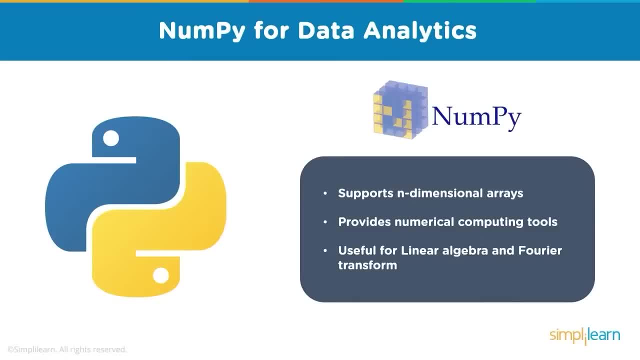 If you want to talk three-dimensional array, you can think of a grid. If you want to talk three-dimensional array, you can think of images. You have your three channels of color, Four if you have an alpha, And then you have your x- y coordinates for the image we're looking at. 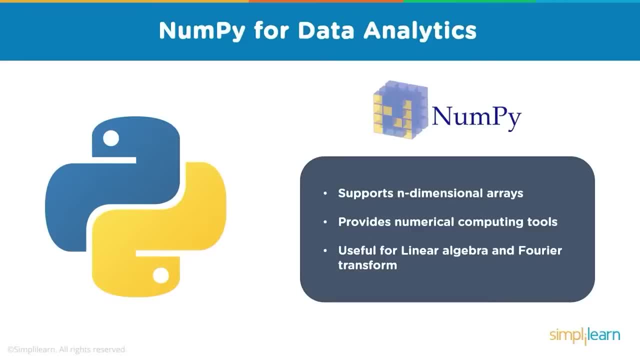 So you can go x, y, and then what are the three channels to generate that color? And NumPy isn't restricted to three dimensions. You can imagine watching a movie. Well, now you have your movie clips and they each have their x number of frames. 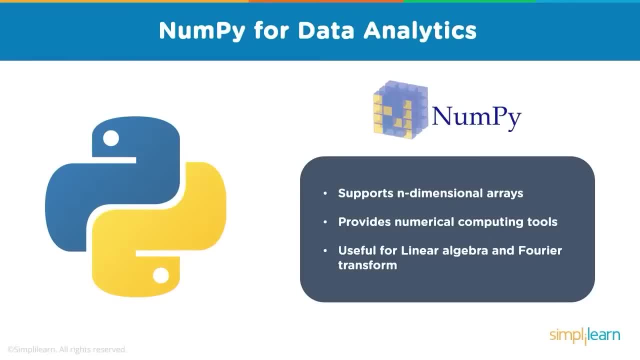 And each of those frames have x, number of x, y coordinates for the pictures in each frame, And then you have your three dimensions for the colors. So NumPy is just a great way to work with n-dimensional arrays. Now, closely with NumPy is Pandas. 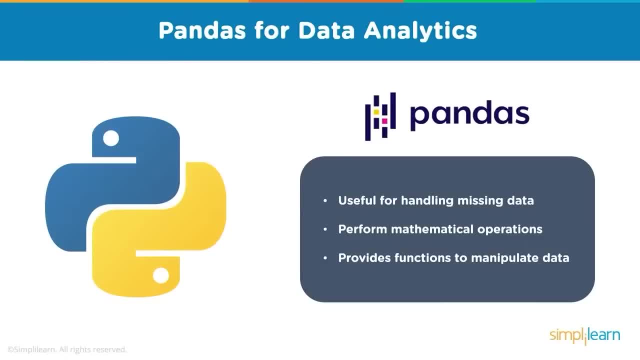 Useful for handling missing data. Perform mathematical operations. Provides functions to manipulate data. Pandas is becoming huge because it is basically a data frame And if you're working with big data and you're working in Spark or any of the other major packages out there, 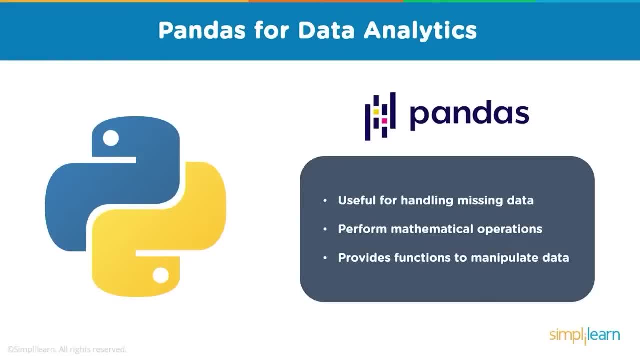 you realize that the data frame is very central to a lot of that And you can look at it as an Excel spreadsheet. You have your columns, You have your rows or indexes And you can do all kinds of different manipulations of the data within. 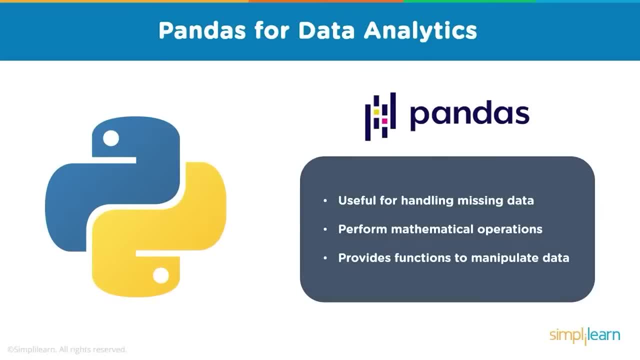 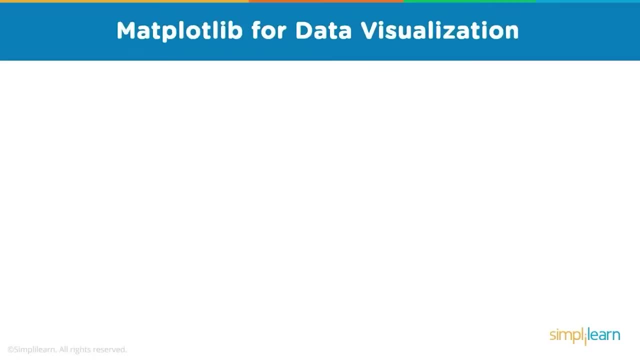 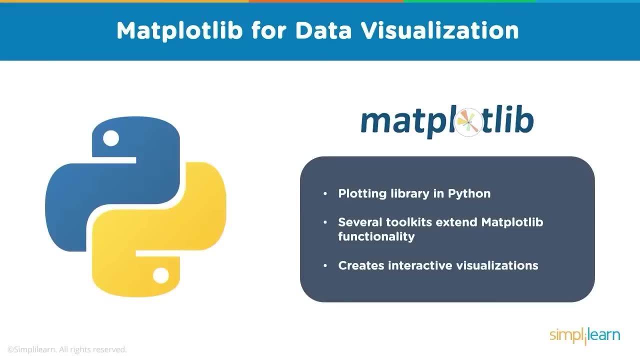 including filling in missing data, which is a big thing when you're dealing with large pools or lakes of data where they might be collected differently from different locations, And Matplot library. We did kick over the SciPy, which is a lot of mathematical computations. 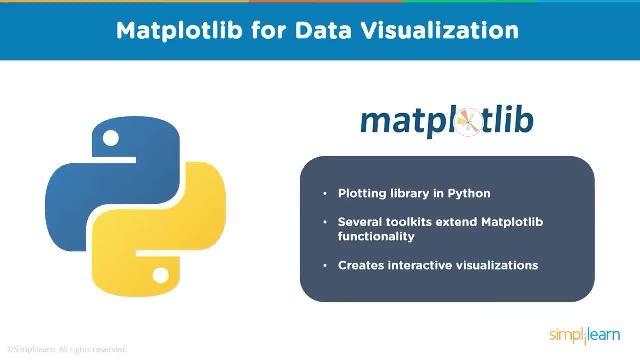 which usually runs in the background of NumPy and Pandas, Although you do use them. they're useful for a lot of other things in there. But the Matplot library. that's the final part. That's what you want to show people. 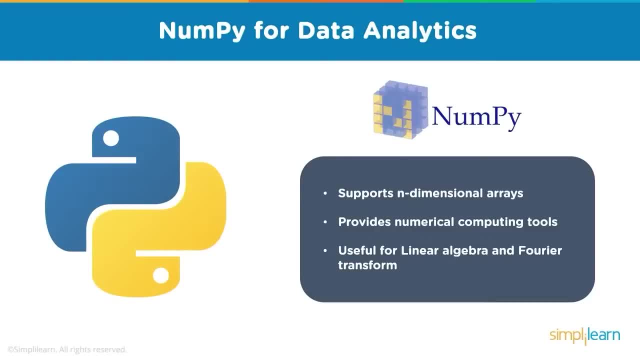 a grid or data, It's not even numbers. It's not even numbers because you can also put words and characters and just about anything into that array, But you can think of a grid and then you can have a grid inside a grid and you end. 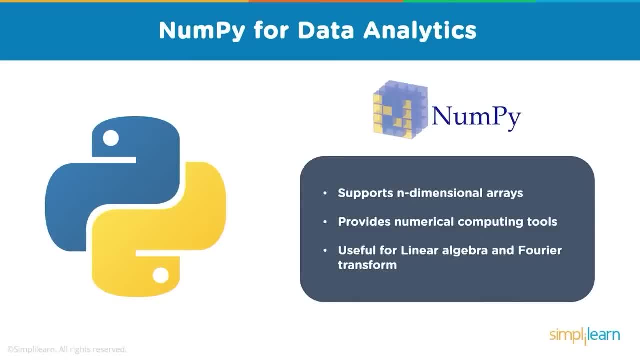 up with a nice three-dimensional array. If you want to talk three-dimensional array, you can think of images. You have your three channels of color, four if you have an alpha, and then you have your x-y coordinates for the image we're looking at. 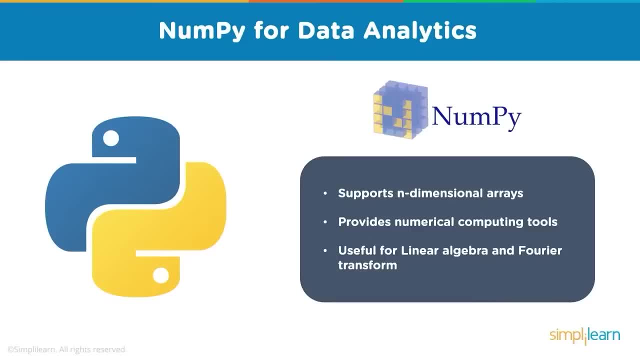 So you can go x, y and then what are the three channels to generate that color? And NumPy isn't restricted to three dimensions. You could imagine Watching a movie. Well, now you have your movie clips and they each have their x number of frames and each. 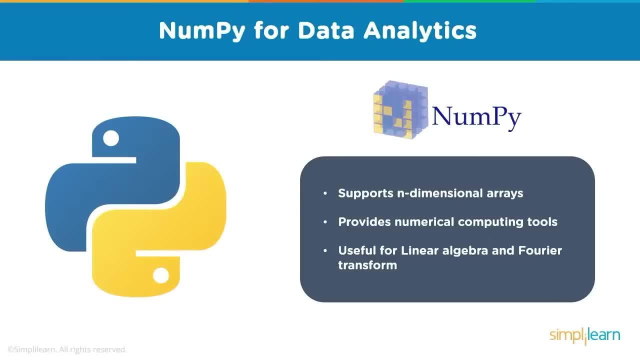 of those frames, have x, number of x, y coordinates for the pictures in each frame, and then you have your three dimensions for the colors. So NumPy is just a great way to work with n-dimensional arrays. Now, closely with NumPy is Pandas. 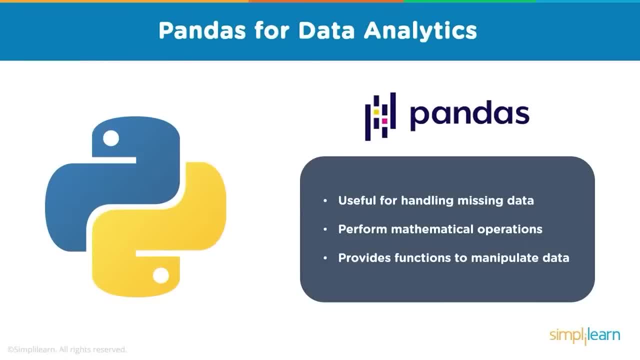 Useful for handling missing data. perform mathematical operations. provides functions to manipulate data. Pandas, Pandas, Pandas, Pandas. Where are those functions called? Well, it goes on. There is a function called NAUive. Now, upon every single function there is. 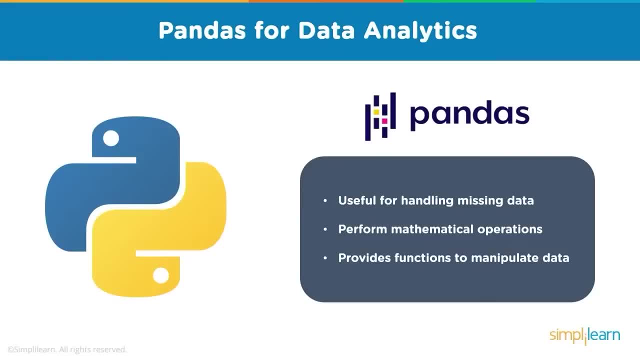 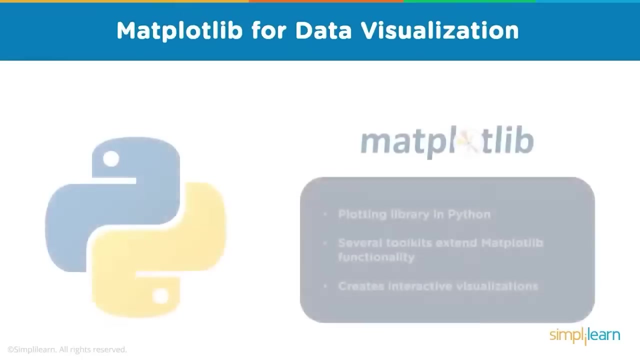 a function called a момент, which bothела 1, is only a second, But I'm about to do something else. Manipulations are very common: file labeling data or lakes of data, where they might be collected differently from different locations. 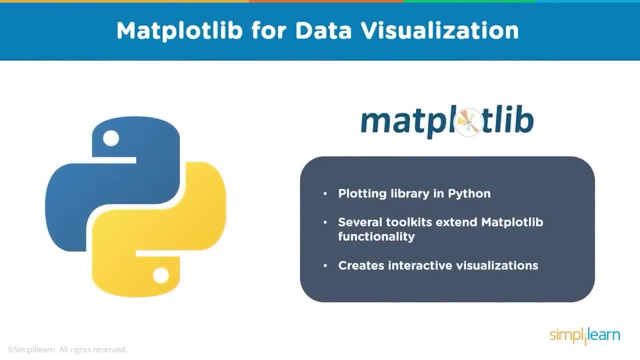 And matplotlib. We did kick over the SciPy, which is a lot of mathematical computations, which usually runs in the background of NumPy and Pandas, Although you do use them, they're useful for a lot of other things in there, But the matplotlib, that's the final part. 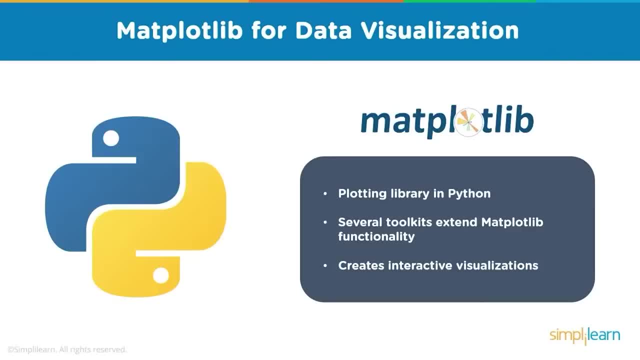 That's what you want to show people And this is your plotting library. in Python, Several toolkits extend matplotlib functionality. There's like 100 different toolkits to extend matplotlib, which range from how to properly display star constellations from astronomy. 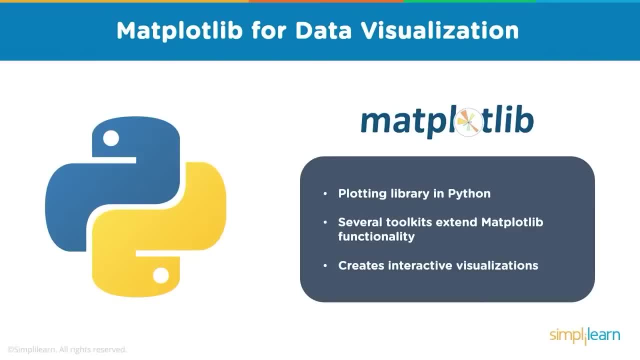 And this is your plotting library in Python. Several toolkits extend Matplot library functionality. There's like a hundred different toolkits to extend Matplot library, which range from how to properly display star constellations from astronomy. There's a very specific one built just for that. 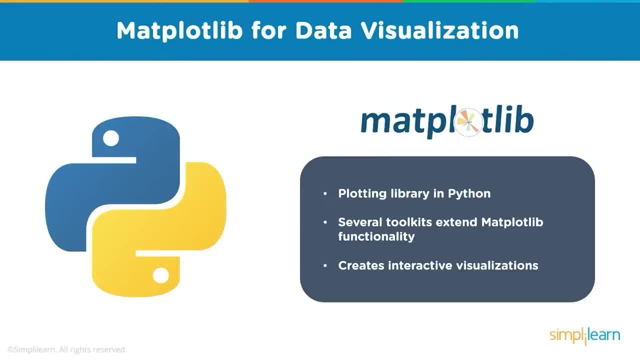 All the way to some very generic ones. We'll actually add Seaborn in when we do the labs in a minute. Several toolkits extend Matplot library functionality and it creates interactive visualization, So there's all kinds of cool things you can do as far as just displaying graphs. 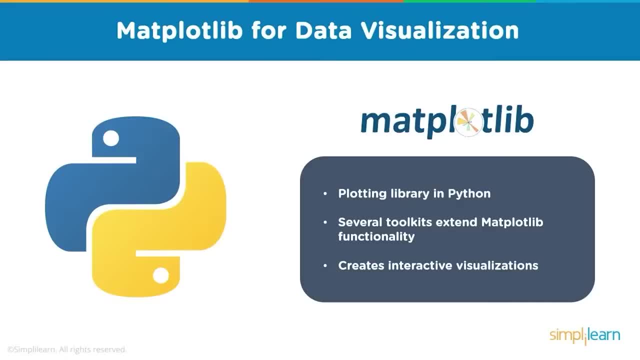 And there's even some that you can create interactive graphs. We won't do the interactive graphs, but you'll see, you'll get a pretty good grasp of some of the different things you can do in Matplot library. Let's jump over to the demo. 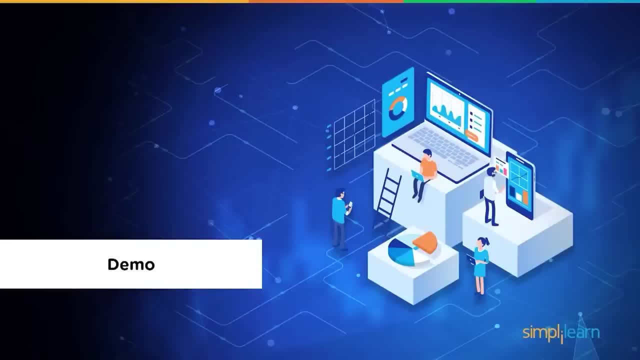 which is my favorite: Roll up our sleeves and get our hands in on what we're doing. Now. there's a lot of options when we're dealing with Python. You can use PyCharm as a really popular one, And you'll see this all over the place. 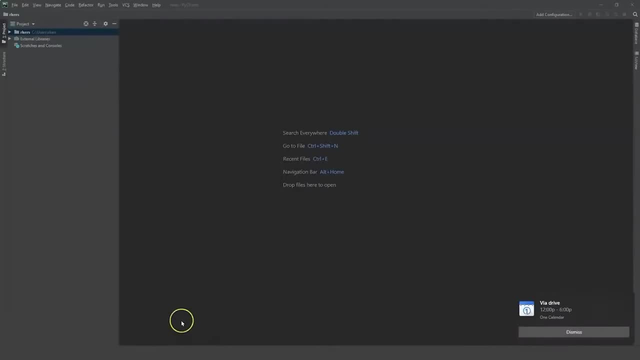 So it's one of the main ones that's out there, And there's a lot of other ones. I used to use NetBeans, which has kind of lost favor. Don't even have it installed on my new computer, But the most popular one right now for data science. 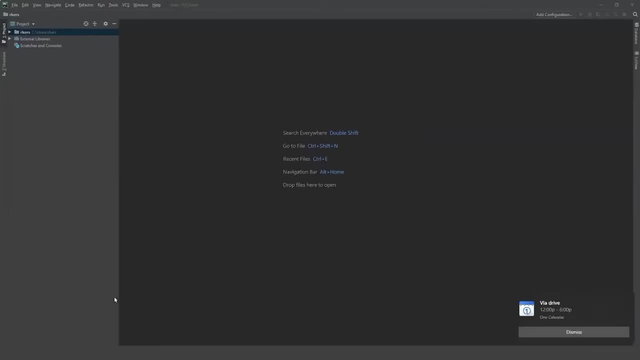 Now PyCharm is really popular for Python, general development, For data science. we usually go to Jupyter, Notebook or Anaconda, And we're going to jump into Anaconda because that's my favorite one to go to, because it has a lot of external tools for us. 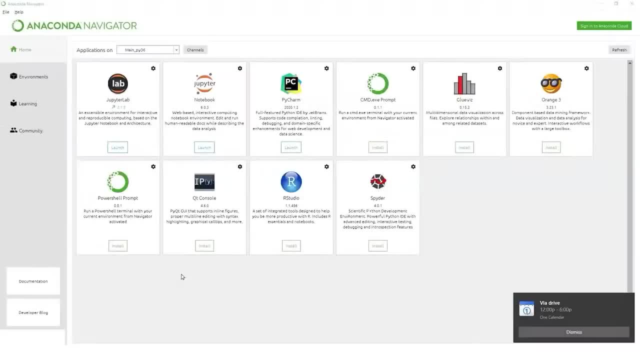 We're not going to dig into those, but we will pop in there so you can see what it looks like. So with Anaconda we have our JupyterLab, We have our Notebook. These are identical. JupyterLab is an upgrade to the Notebook with multiple tabs. 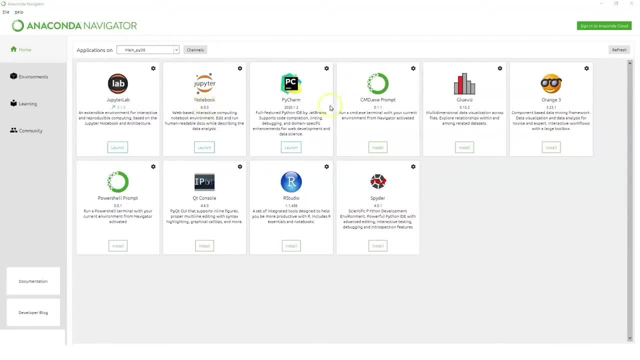 That's all it is, And we'll be using the Notebook, And you can see that PyCharm is so popular with Python that we even have it highlighted here in Anaconda as part of the setup. Jupyter Notebook can also be a standalone. 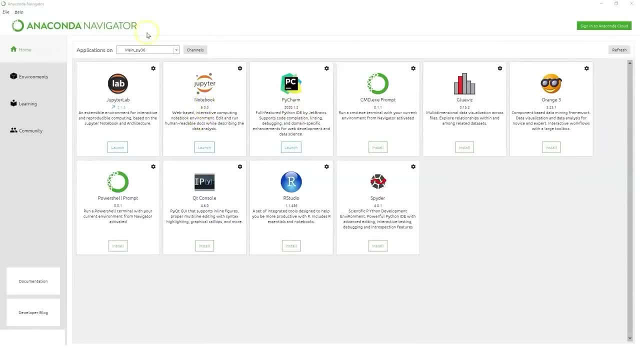 So we're actually going to be running Jupyter Notebook And then you have your different environments I have we're going to be under mainPy3.6.. There's a root one And I usually label it Py3.6.. 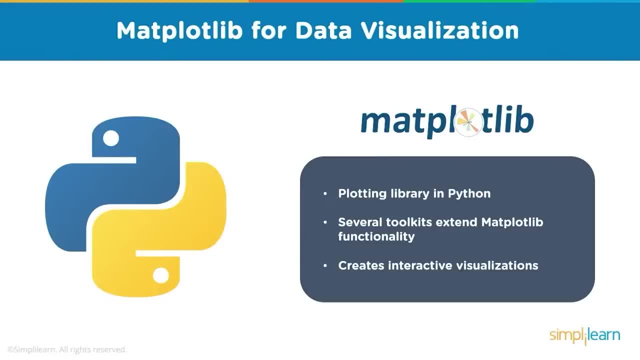 There's a very specific one built just for that, all the way to some very generic ones. We'll actually add Seaborn in when we do the labs in a minute. Several toolkits extend matplotlib functionality and it creates interactive visualization. So there's all kinds of cool things. 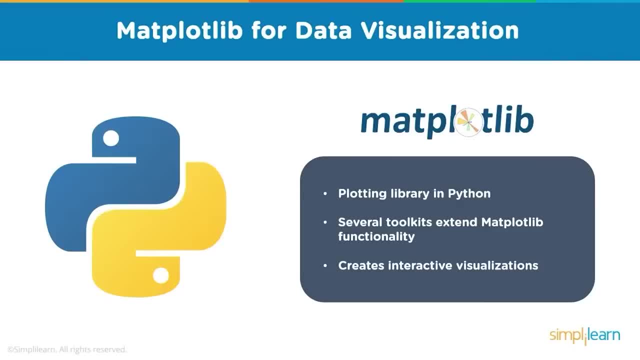 you can do as far as just displaying graphs, And there's even some that you can create interactive graphs. We won't do the interactive graphs but you'll see, you'll get a pretty good grasp of some of the different things you can do in matplotlib library. 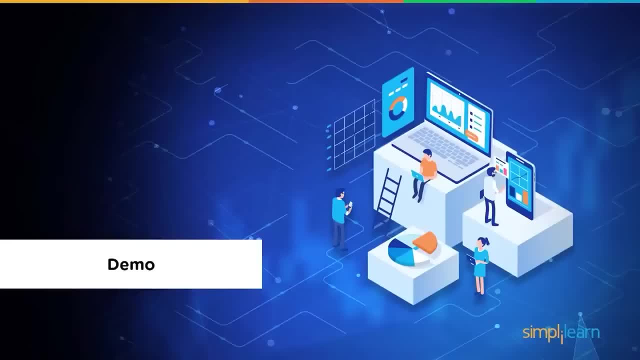 Let's jump over to the demo, which is my favorite. Roll up our sleeves and get our hands in on what we're doing. Now. there's a lot of options when we're dealing with Python. You can use PyCharm as a really popular one. 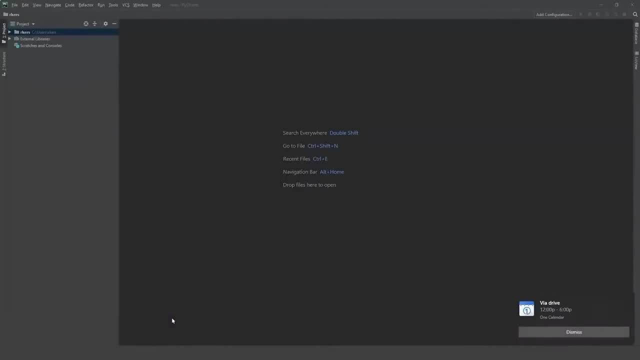 And you'll see this all over the place. So it's one of the main ones that's out there, And there's a lot of other ones. I used to use NetBeans, which has kind of lost favor. Don't even have it installed on my new computer. 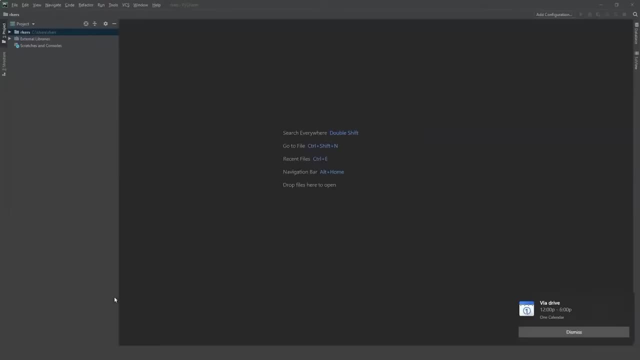 But the most popular one right now for data science. Now PyCharm's really popular for Python general development. For data science we usually go to Jupyter, Notebook or Anaconda, And we're going to jump into Anaconda because that's my favorite one to go to. 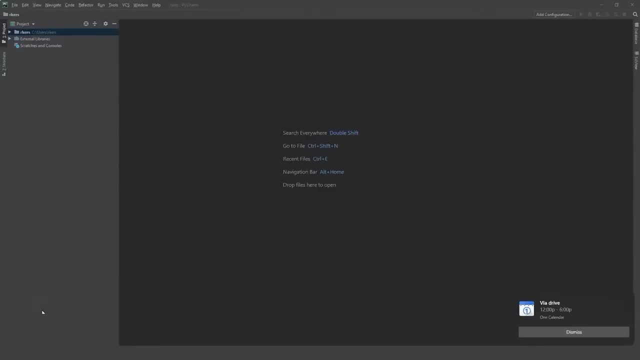 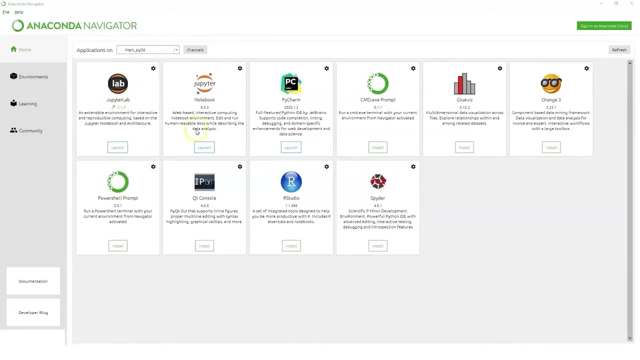 because it has a lot of external tools for us. We're not going to dig into those, but we will pop in there so you can see what it looks like. So with Anaconda, we have our JupyterLab, We have our notebook. 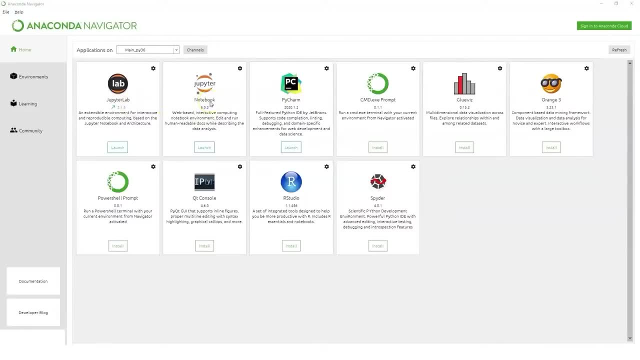 These are identical. JupyterLab is an upgrade to the notebooks with multiple tabs. That's all it is, And we'll be using the notebook. And you can see that PyCharm is so popular with Python that we even have it highlighted here in Anaconda. 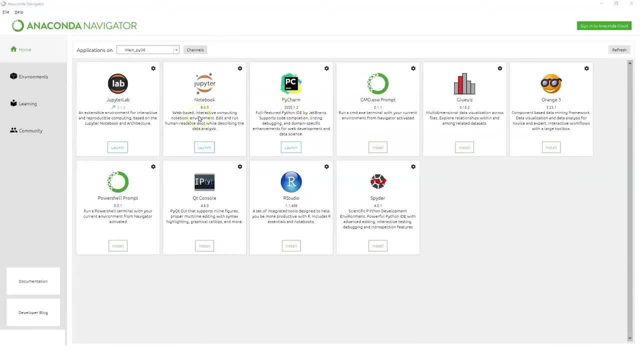 as part of the setup, Jupyter Notebook can also be a standalone. So we're actually going to be running Jupyter Notebook And then you have your notebook And, in very different environments, we're going to be under main Pi 3.6.. 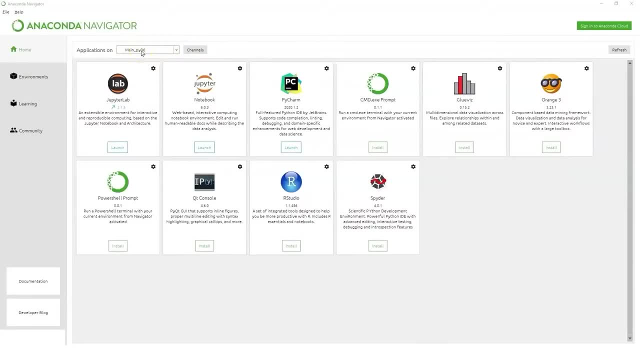 There's a root one And I usually label it Pi 3.6.. The reason is currently, as of writing, this TensorFlow only works in 3.6 and not in 3.7 or 3.8 for doing neural networks. 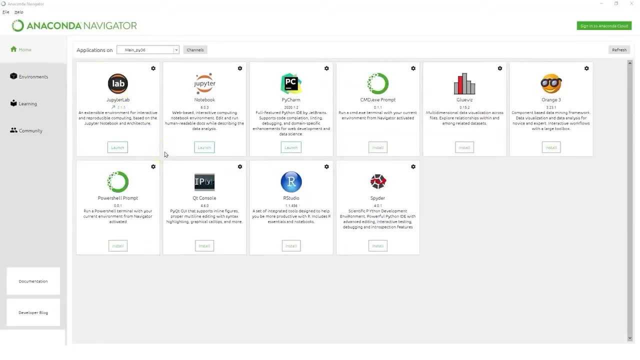 But you can actually have multiple environments, which is nice. They separate the kernels, so it helps protect your computer when you're doing development, And this is just a great way to do a display or a demo, especially if you're looking for that job. 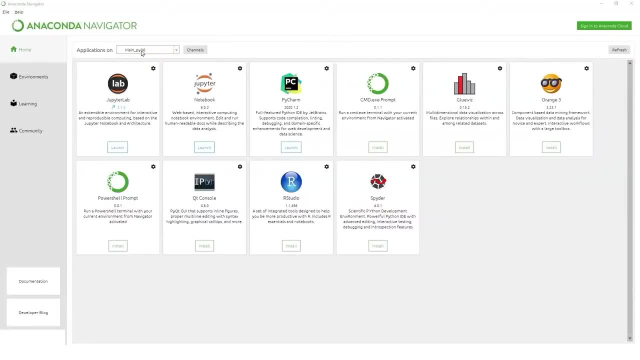 The reason is is currently, as of writing this, TensorFlow only works in 3.6 and not in 3.7 or 3.8 for doing neural networks, But you can actually have multiple environments, which is nice They're. they separate the kernels. 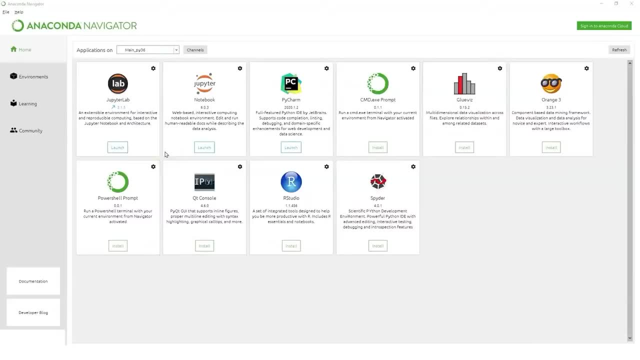 so it helps protect your computer when you're doing development, And this is just a great way to do a display or a demo, especially if you're looking for that job. Pull up your laptop, open it up, Or if you're doing a meeting. 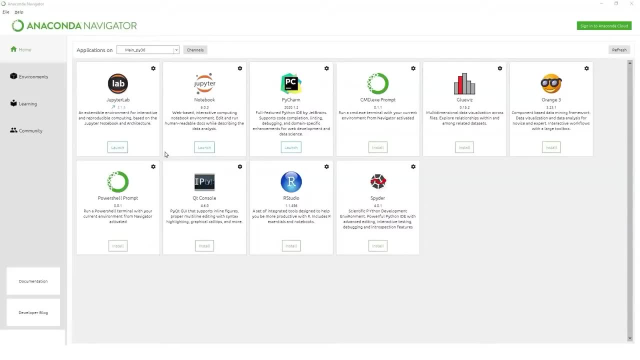 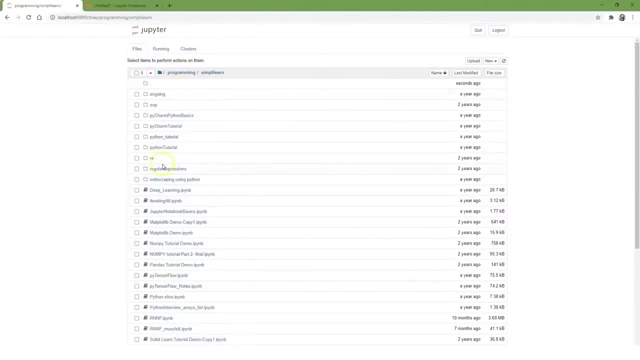 get it broadcast up to the big screen so that the CEO can see what you're looking at. And when we launched the Notebook, it actually opens up a file browser. in whatever web browser you have- This happens to be Chrome- And then you can just go under new. 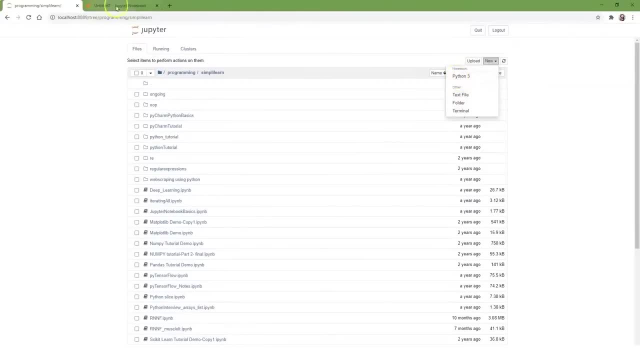 There's a lot of different options depending on what you have installed- Python 3.. And this just creates an untitled version of this And you can see here I'm actually in a Simply Learn folder for other work I've done for Simply Learn. 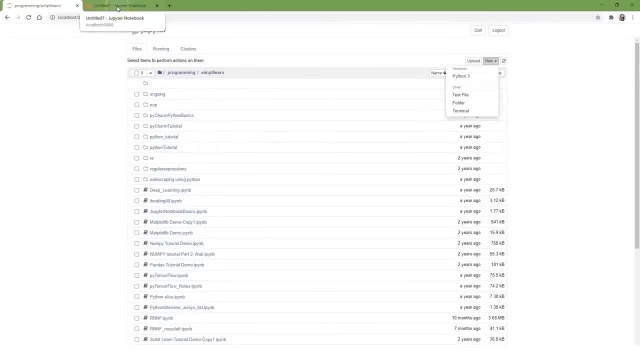 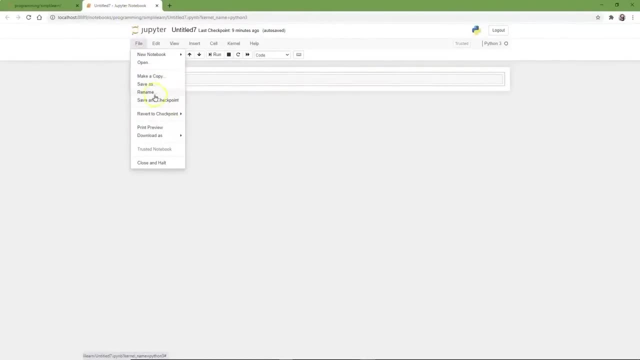 And that's where I save all my stuff and I can browse through other folders, making it real easy to jump from one project to another. And under here we'll go ahead and change the name of this and we'll go ahead and rename it. 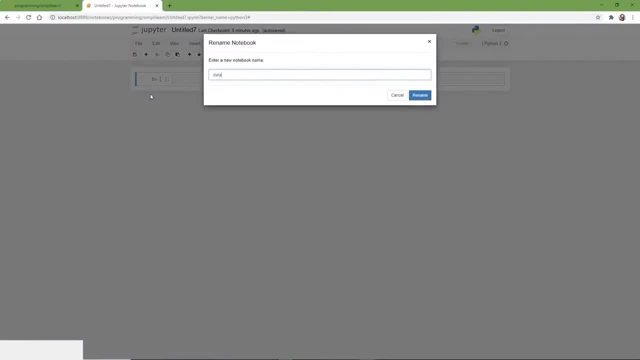 Data Analytics. Data Analytics- Just so I can remember what I was doing, Which is probably about 50 of the folders in here or files in here right now. So let's go ahead and jump in there and take a look at some of these different tools. 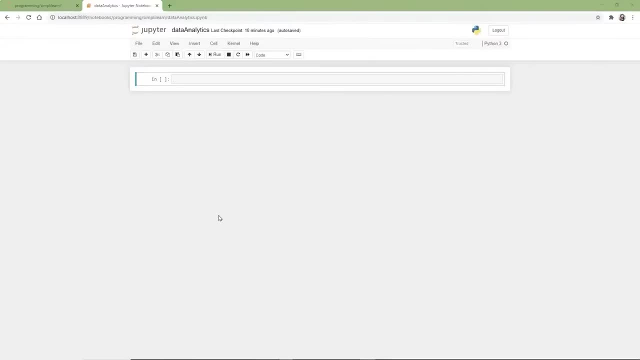 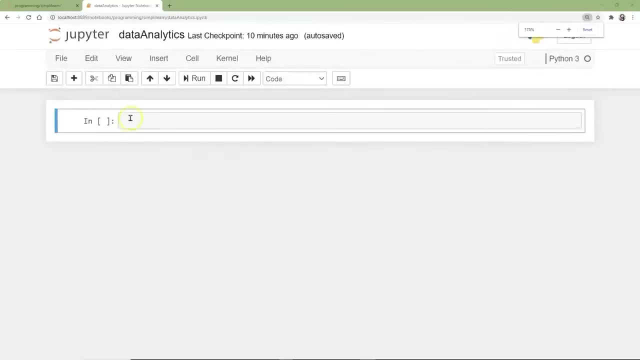 that we were looking at. And as we go through the demo, let's start with the numpy, the least visually exciting, And I'm going to zoom in here so you can see what we're doing. And the first thing we want to do is import numpy. 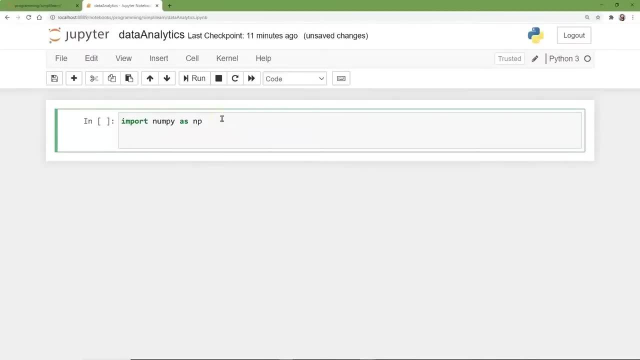 And we'll import it as np. That is the most common numpy terminology And let's go ahead and change the view. so we also have the line numbers. I don't know why we probably won't need them, but I like it for easy reference. 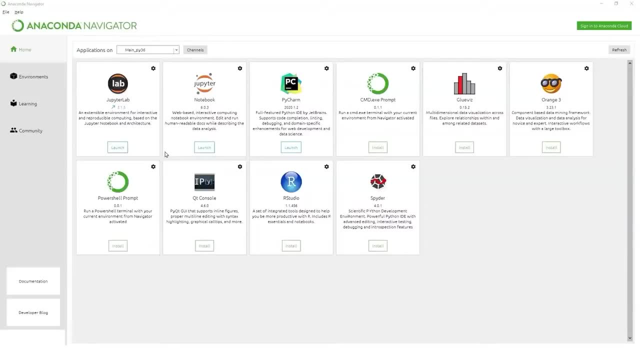 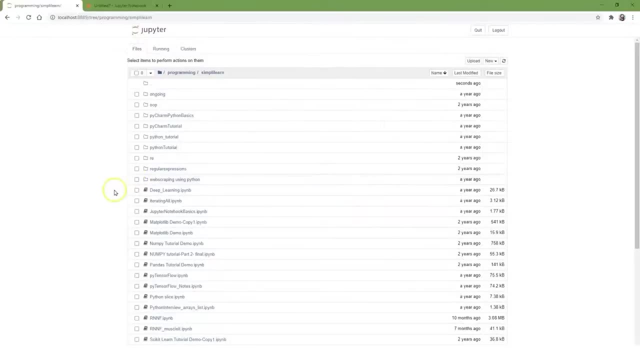 Pull up your laptop, Open it up, Or, if you're doing a meeting, get it broadcast up to the big screen so that the CEO can see what you're looking at. And when we launch the notebook, it actually opens up a file browser in whatever web browser you have. 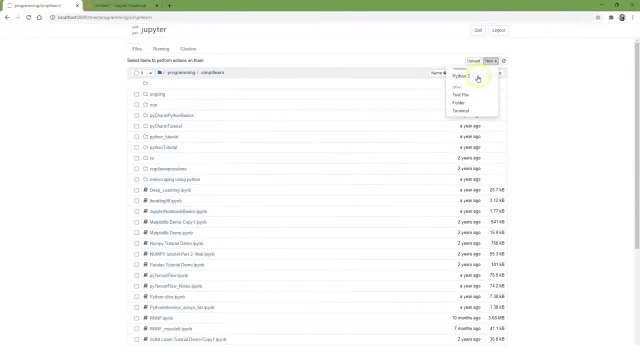 This happens to be Chrome, And then you can just go under New. There's a lot of different options depending on what you have installed, Python 3.- And this just creates an untitled version of this, And you can see here I'm actually. 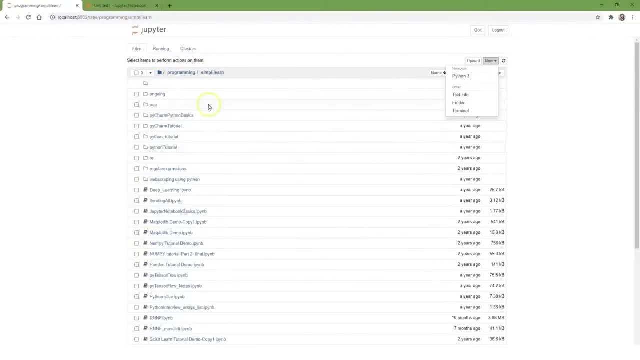 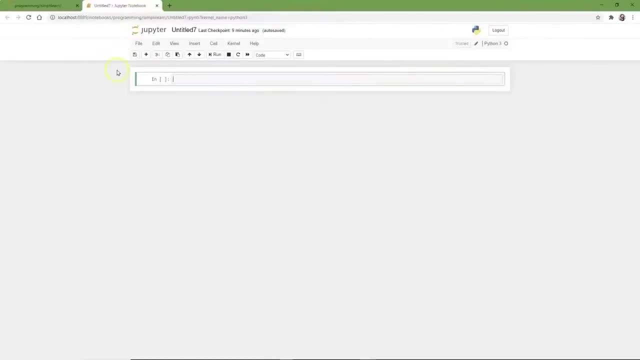 in a Simply Learn folder for other work I've done for Simply Learn And that's where I save all my stuff And I can browse through other folders, making it real easy to jump from one project to another. And under here we'll go ahead and change the name of this. 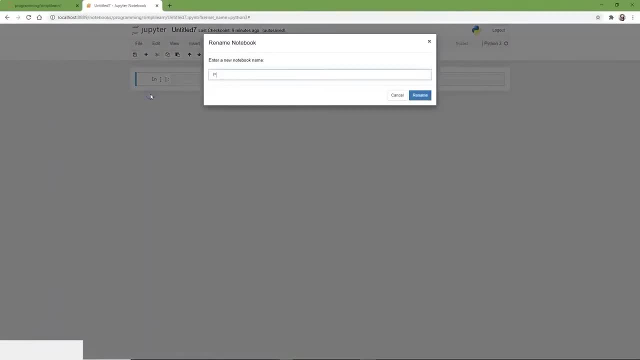 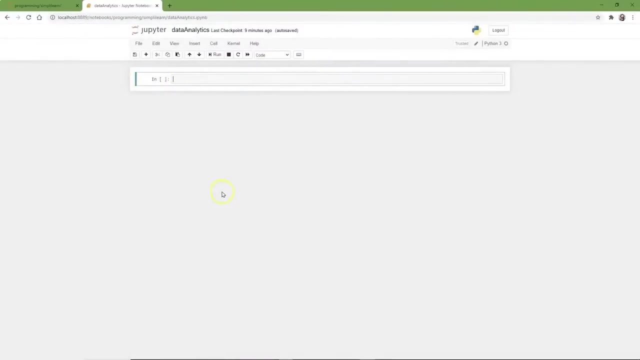 And we'll go ahead and rename it Data Analytics. Data Analytics- Just so I can remember what I was doing, which is probably about 50 of the folders in here or files in here right now, So let's go ahead and jump in there. 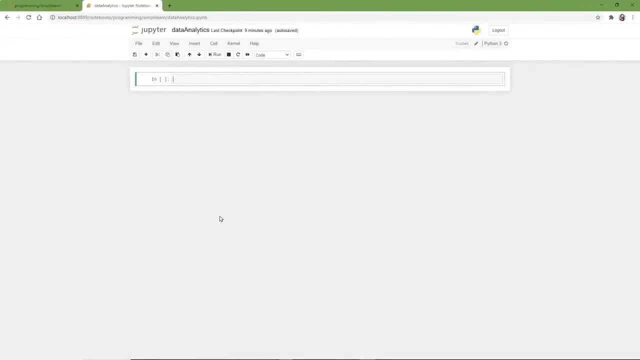 and take a look at some of these different tools. So we were looking at And, as we go through the demo, let's start with the NumPy, the least visually exciting, And I'm going to zoom in here so you can see what we're doing. 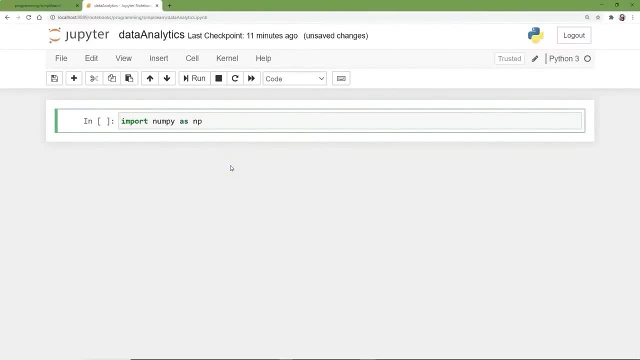 And the first thing we want to do is import NumPy, And we'll import it as NP. That is the most common NumPy terminology, And let's go ahead and change the view so we also have the line numbers. I don't know why. 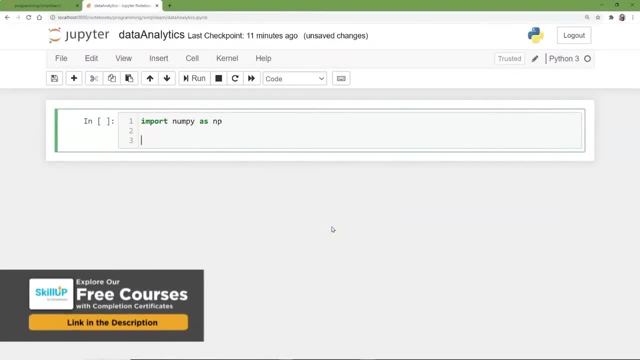 We probably won't need them, But I like it for easy reference. And then we'll create a one-dimensional array. We'll just call this array1.. And it equals nparray, And you put your array information in here. In this case, we'll spell it out. 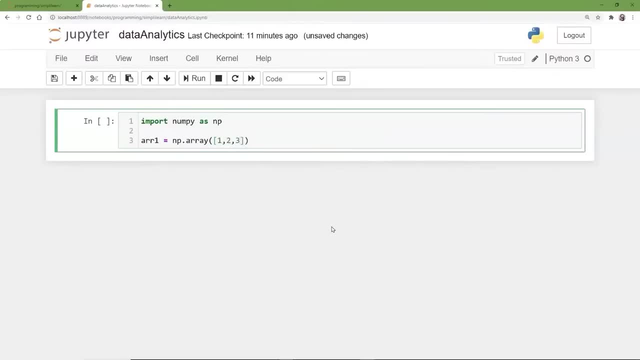 You can actually do a range and other ways. There's lots of ways to generate these arrays, But we'll just do 1,, 2, 3,, so three integers, And if we print our array1, we can go ahead and run this. 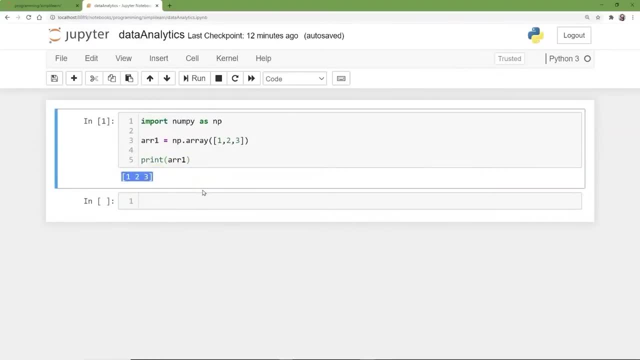 And you can see right here it prints 1,, 2, 3.. You can see why this is a really nice interface to show other people what you're doing with the Jupyter Notebook. So this is the basic. We've created an array. 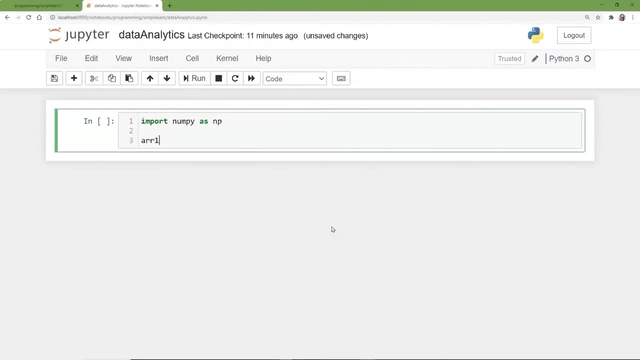 And then we'll create a one-dimensional array. We'll just call this array1.. And it equals nparray, And you put your array information in here. In this case, we'll spell it out. You can actually do like a range and other ways. 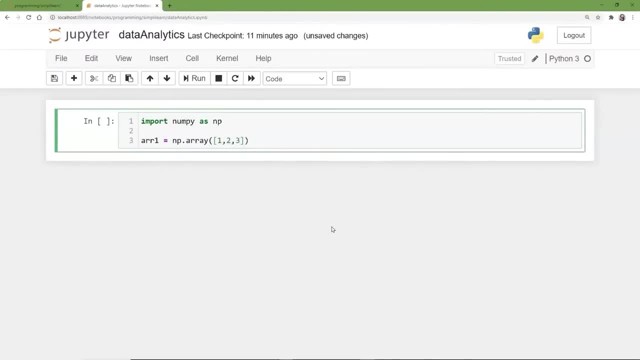 There's lots of ways to generate these arrays, But we'll just do 1,, 2, 3.. So three integers. And if we print our array1, we can go ahead and run this And you can see right here: it prints 1,, 2, 3.. 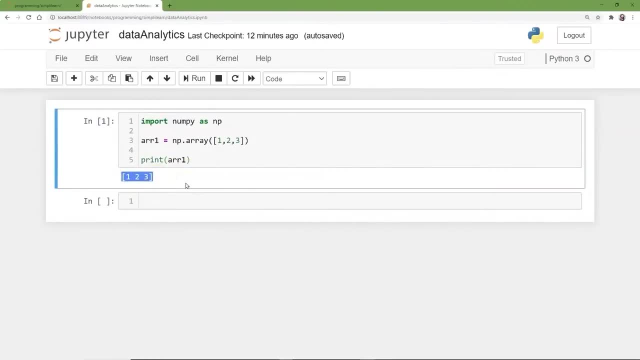 You can see why. this is a really nice interface to show other people what you're doing with the Jupyter Notebook. So this is the basic. We've created an array. This is a one-dimensional array, And then there's the numpy And the array is 1,, 2,, 3.. 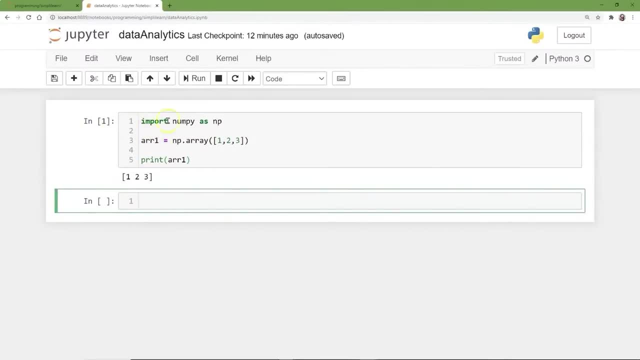 One of the nice things about the Jupyter Notebook is whatever ran in this first setup is still running. It's still in the kernel, So it still has the numpy imported as np And it still has our variable arr1 for array1 equal to nparray of 1,, 2,, 3.. 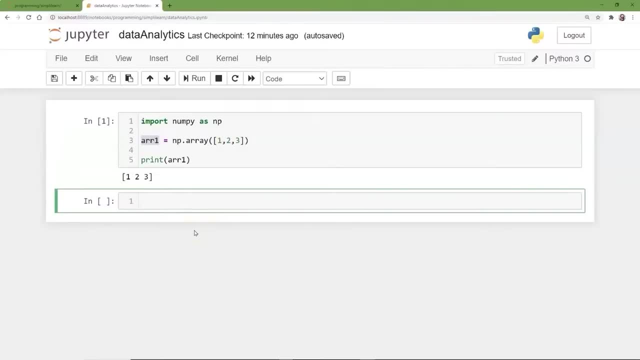 So when we go to the next cell we can check the type of the array We're just going to print. We say, hey, what is this setup in here? And we want type. And then we want: what is the type of array1?. 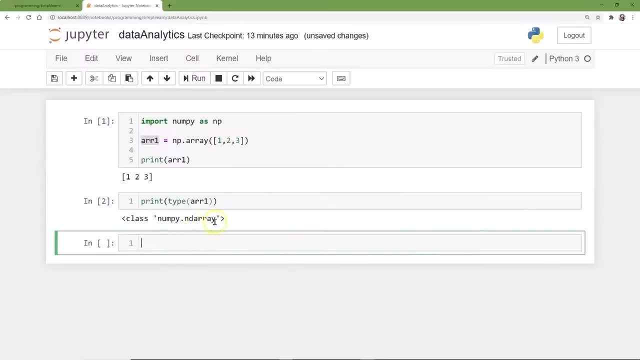 And let's go ahead and run that And it says class numpy ndarray, So it's its own class. That's all we're doing is checking to see what that class is. And if you look at the array class, probably the biggest thing you do- 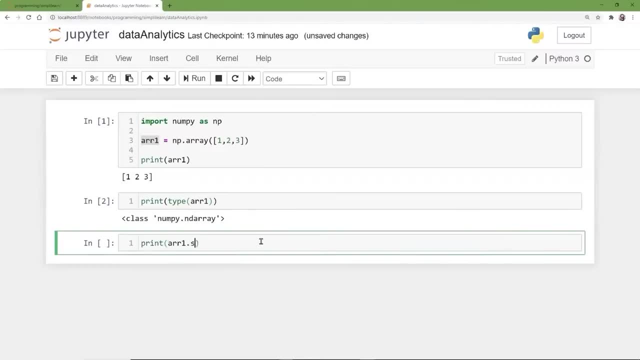 I don't know how many times I find myself doing this, because I forget what I'm working on and I forget I'm working with a three-dimensional or a four-dimensional array And I have to reformat somehow so it works with whatever other things I have. 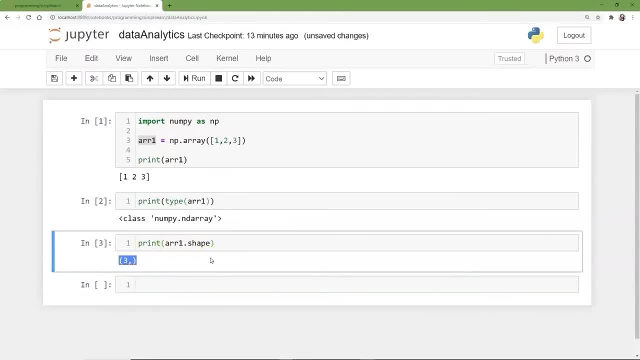 And so we do the array shape. The array shape is just three because it has three members and it's a one-dimensional array. That's all that is, And with the numpy array we can easily access. stick with the print statement If you actually put a variable in Jupyter Notebook. 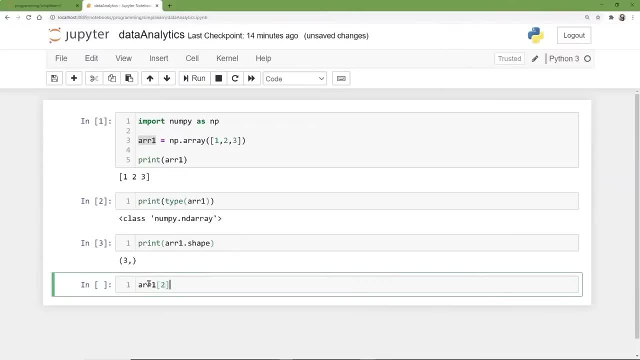 and it's the last one in the cell, it will be the same as a print statement. So if I do this, where array one of two it's the same as doing print array of two. Those are identical statements in our Jupyter Notebook. 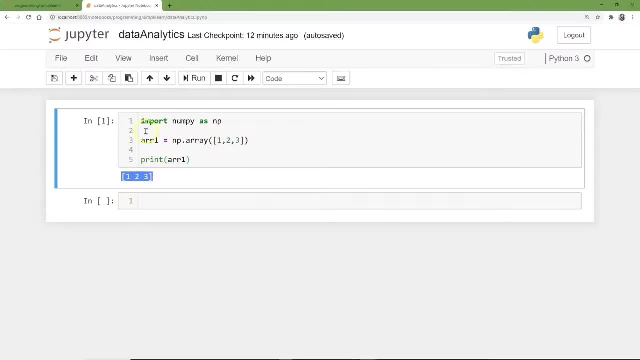 This is a one-dimensional array And then the array is 1,, 2,, 3.. One of the nice things about the Jupyter Notebook is whatever ran in this first setup is still running. It's still in the kernel, So it still has the NumPy imported as NP. 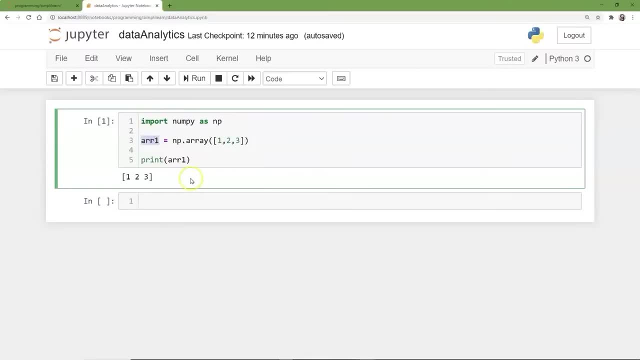 And it still has our variable arr1 for array1, equal to nparray of 1,, 2, 3.. So when we go to the next cell we can check the type of the array We're just going to print. We say, hey, what is this setup in here? 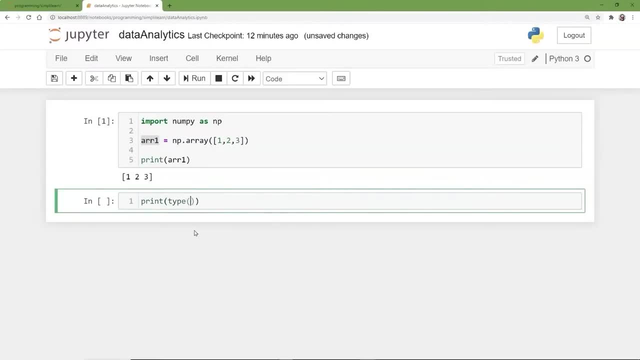 And we want type, And then we want what is the type of array1?. Let's go ahead and run that And it says class NumPy ndarray. So it's its own class. That's all we're doing is checking to see what that class is. 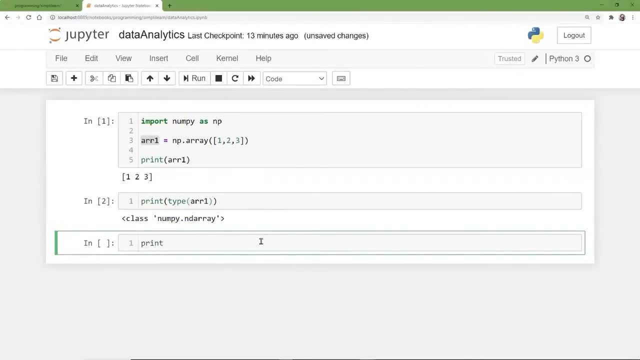 And if you look at the array class, probably the biggest thing you do. I don't know how many times I find myself doing this because I forget what I'm working on And I forget I'm working with a three-dimensional or four-dimensional. 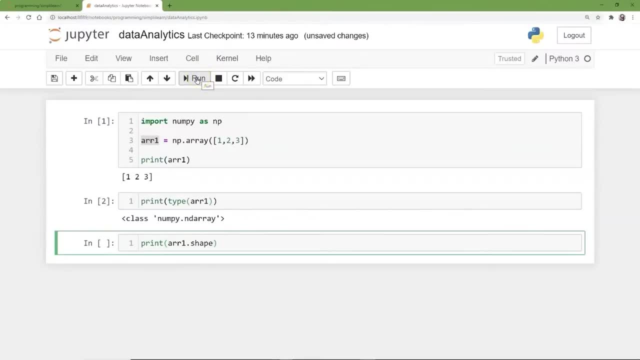 array And I have to reformat somehow so it works with whatever other things I have, And so we do the array shape. The array shape is just three because it has three members And it's a one-dimensional array. That's all that is. 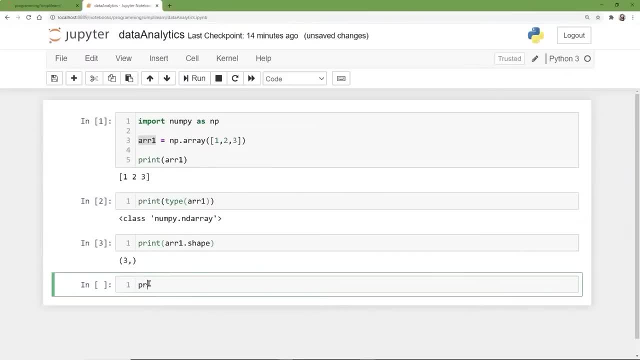 And with the NumPy array we can easily access, stick with the print statement. If you actually put a variable in Jupyter Notebook and it's the last one in the cell, it will be the same as a print statement. So if I do this, where array1 of 2, it's the same as doing print array of 2.. 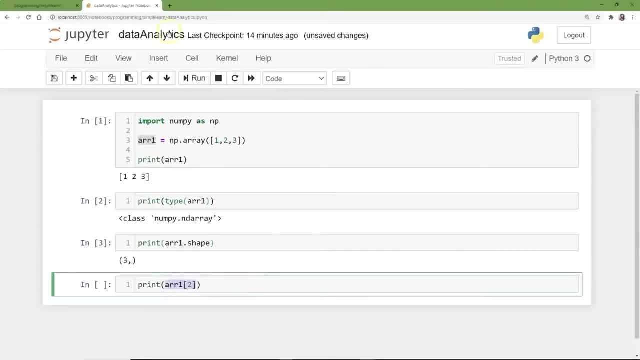 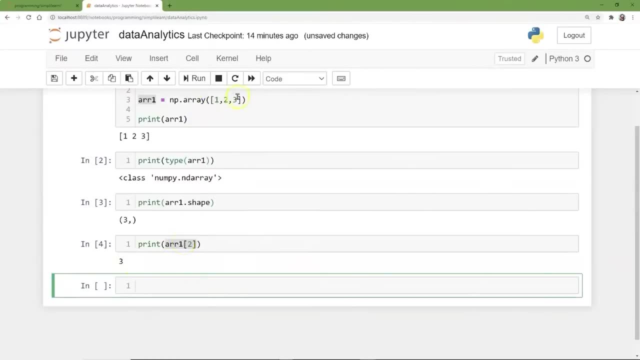 Those are identical statements in our Jupyter Notebook. We'll go and stick with the print on this one, And it's 3.. So there's our print: space 2. And we have 0,, 1,, 2,. 2 equals 3.. 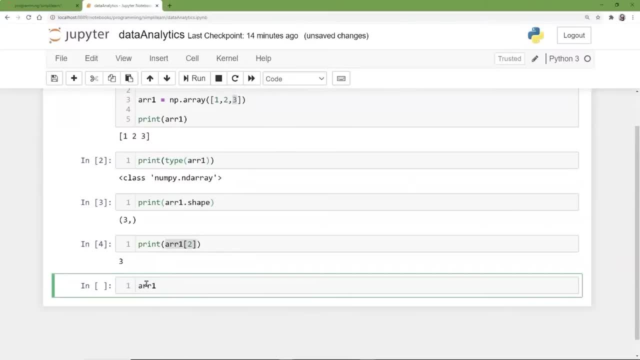 We can easily change that. So we have array1 of place 2 equals 5.. And then if we print our array1, you can see right down here when it comes out: it's 1,, 2, and 5.. 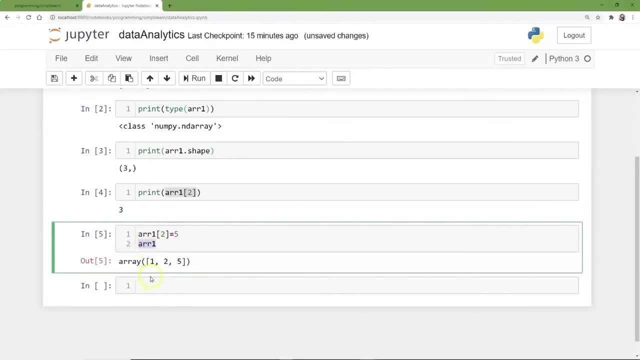 And there I left the print statement off because it's the last variable in the list And it'll always print the variable. if you just put it in like that, That's a Jupyter Notebook thing. Don't do that in PyCharm. 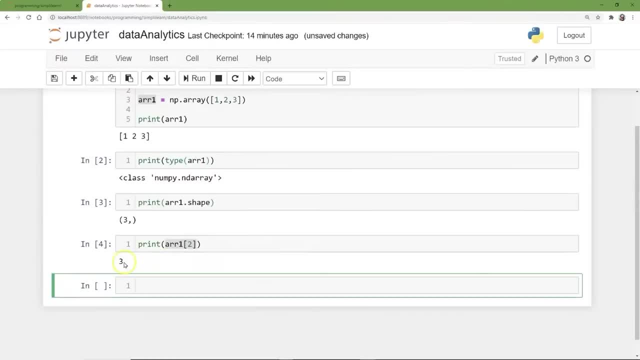 We'll go and stick with the print on this one And it's three. So there's our print. space two And we have zero one. two. Two equals three. We can easily change that. So we have array one of place. two equals five. 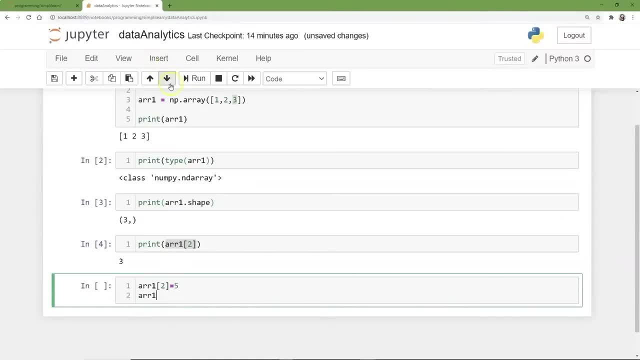 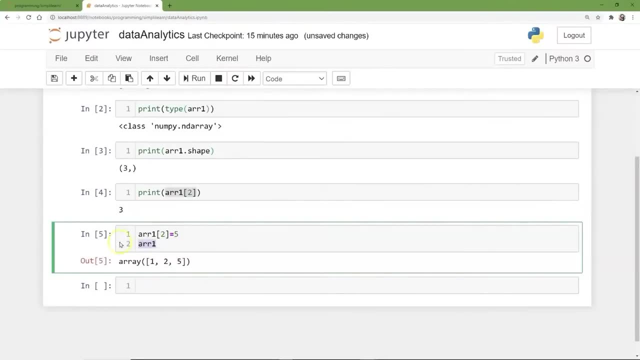 And then if we print our array one, you can see right down here when it comes out, it's one, two and five, And there I left the print statement off because it's the last variable in the list. It will always print the variable. 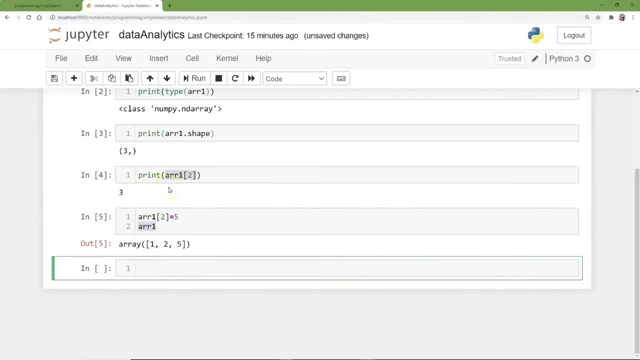 if you just put it in like that, That's a Jupyter Notebook thing. Don't do that in PyCharm. I've forgotten before doing a demo And we talked about multiple dimensions, So we'll do an array, two-dimensional array. 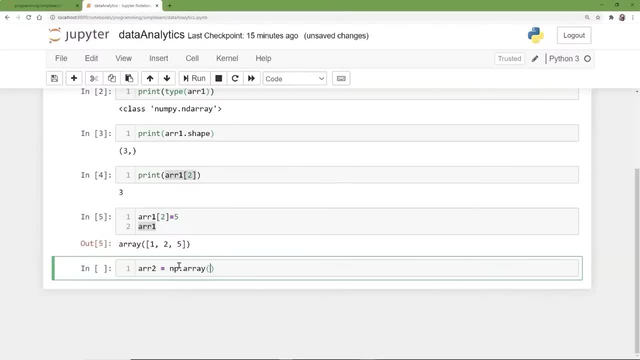 And this is again a numpy array, And in the numpy array we need our first dimension- We'll do one, two, three- And our second dimension- three, four, five. And you can see right here that when we hit the 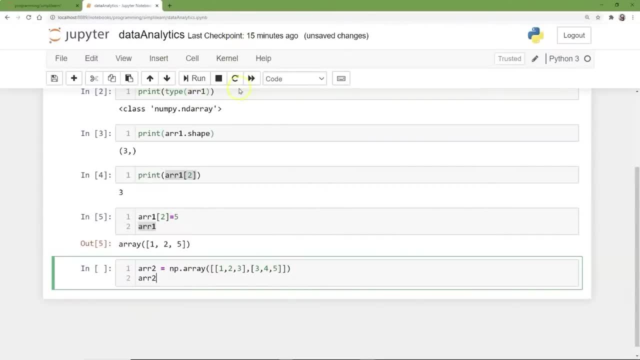 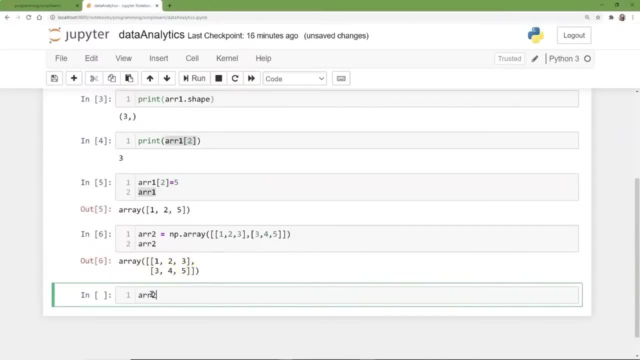 we'll do this. We'll just do array two And we can run that, And there's our array two. one, two, three, three, four, five. We can also do array two of one, And then we can do. 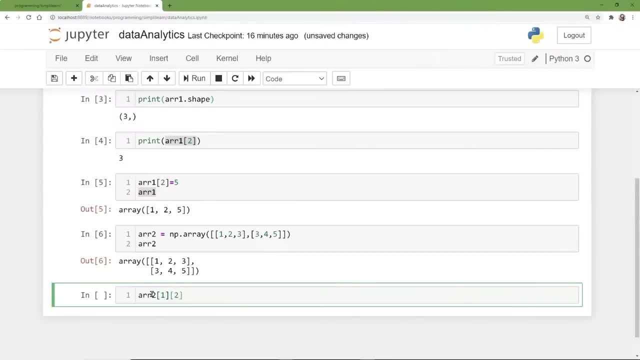 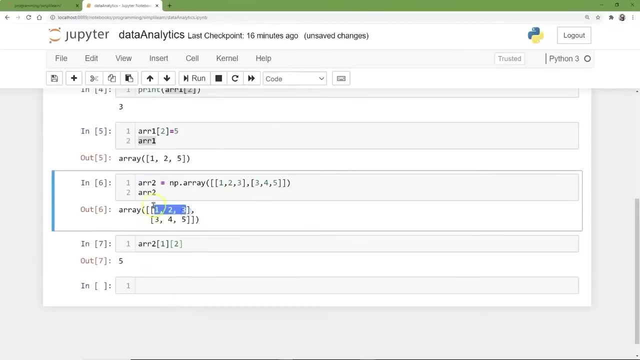 let's do zero. It doesn't really matter which one. Actually, let's do two. There we go, And if I run this, it'll print out five, Because here we are. This is zero, Zero. one, two, three. 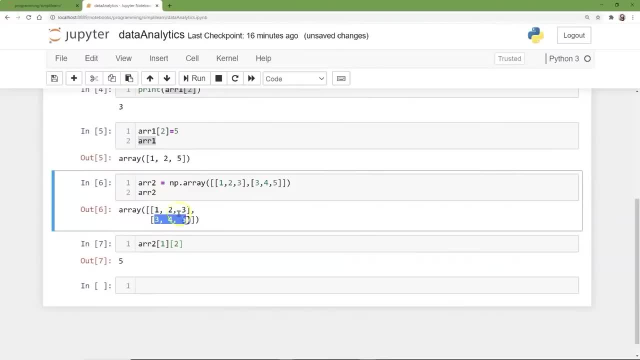 is on our zero row, Three, four, five is on our one row And we start with zero And then the two, zero one. two goes to the five, And then maybe we forgot what we were working with, So we'll go do array two dot shape. 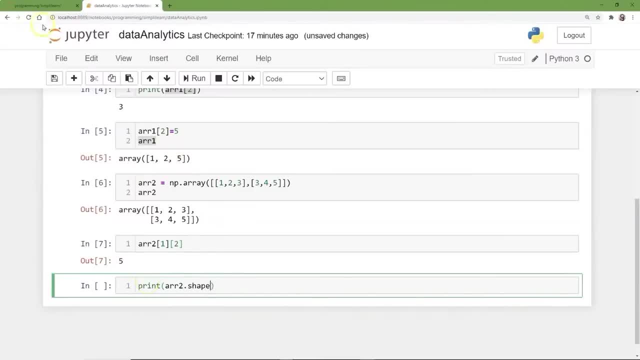 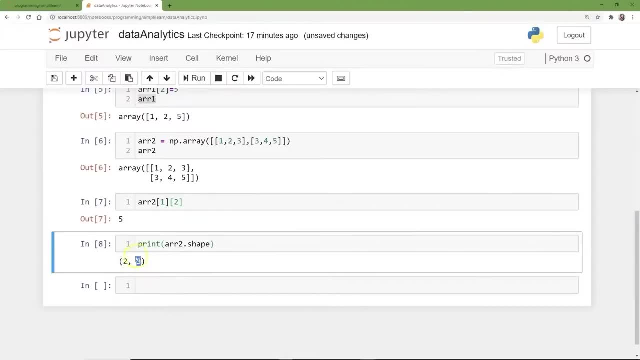 And if we do array two of shape, we'll go and run that, We'll see we have two rows and each row has three elements: Two dimensional array, Two, three. If you looked up here when we did it before, it just had three comma, nothing. 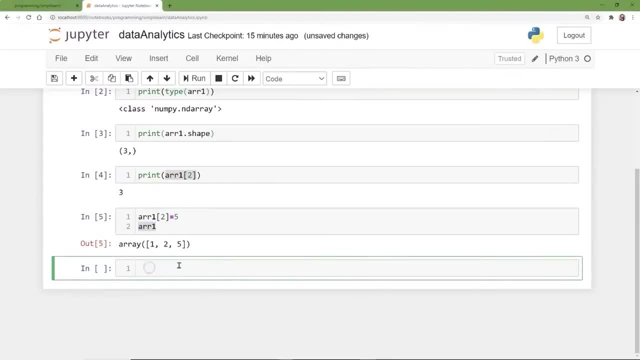 I've forgotten before doing a demo, And we've talked about multiple dimensions. So we'll do an array, two-dimensional array, And this is again a NumPy array, And in the NumPy array we need our first dimension. 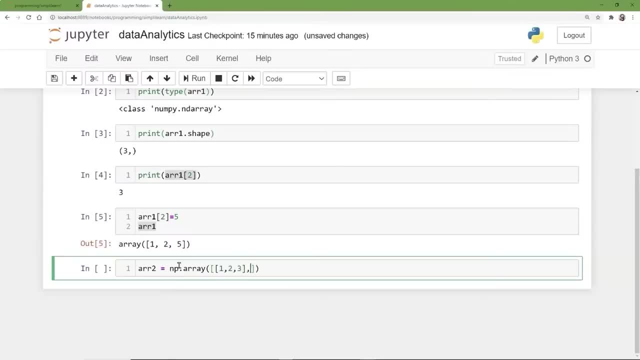 We'll do 1,, 2,, 3.. And our second dimension, 3,, 4,, 5.. And you can see right here that when we hit the, we'll do this, We'll just do array2.. And we can run that. 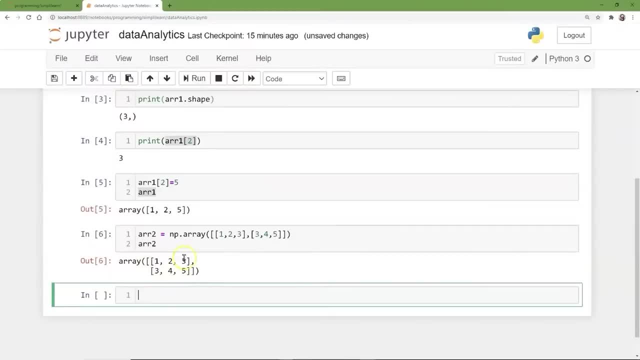 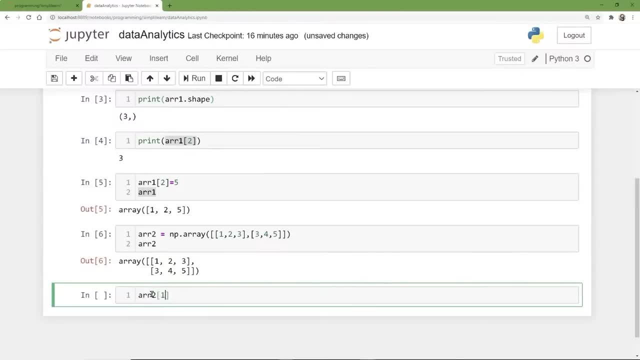 And then we can do: let's do 0.. It doesn't really matter which one Actually. let's do 2.. There we go, And if I run this, it'll print out 5.. Because here we are, This is 0.. 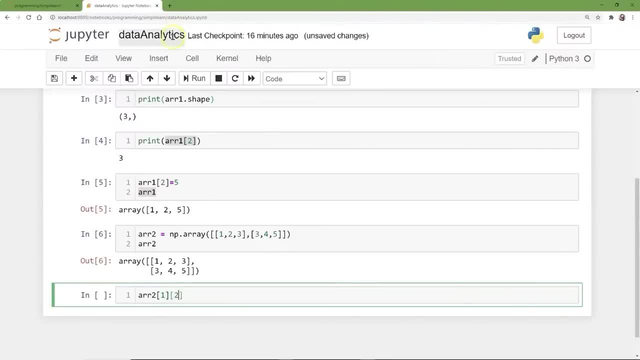 0,, 1,, 2,, 3 is on our 0 row. 3,, 4,, 5 is on our 1 row And we start with 0.. And then the 2.. 0,, 1,, 2,, 3 is on our 0 row. 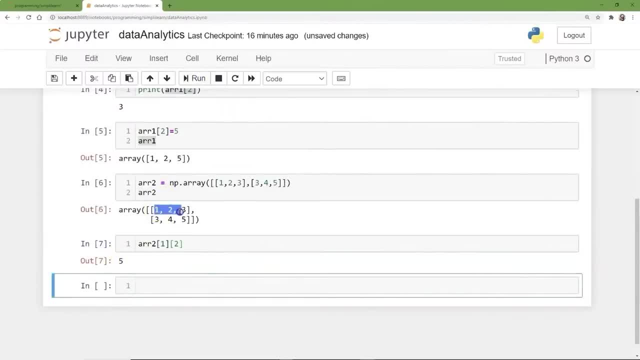 3,, 4,, 5 is on our 1 row And we start with 0.. And then the 2.. 0, 1,, 2, 3 is on our 0 row. 0, 1,, 2, 3 is on our 0 row. 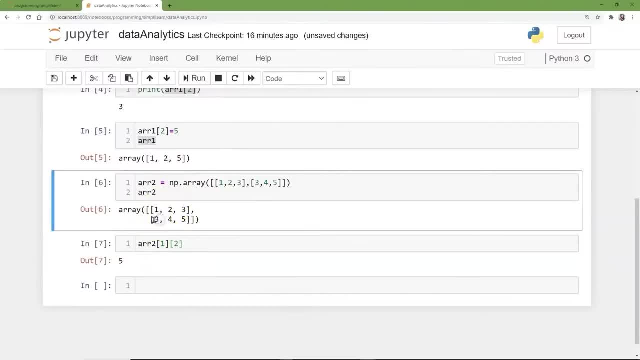 3,, 4, 5 is on our 1 row And we start with 0. And then the 2.. 0,, 1, 2 goes to the 5.. And then maybe we forgot what we were working with. 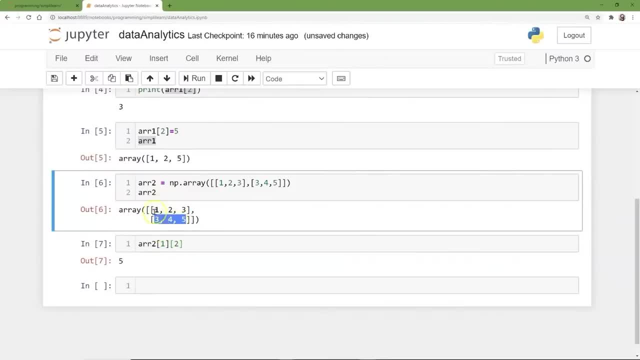 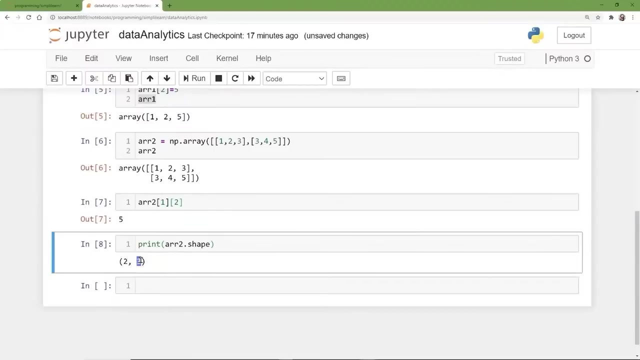 So we'll go do array2.shape And if we do array2 of shape we'll go and run that. We'll see, we have two rows And each row has 3 rows, 3 elements, 2 dimensional array 2, 3.. 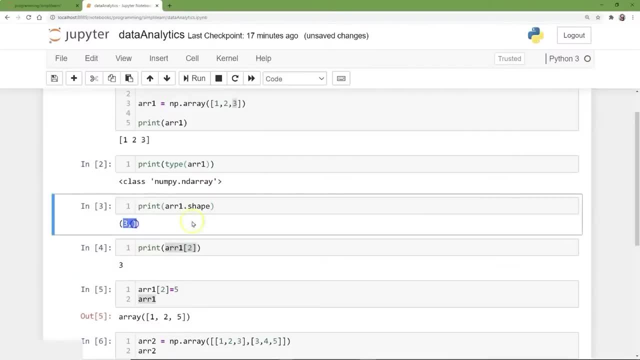 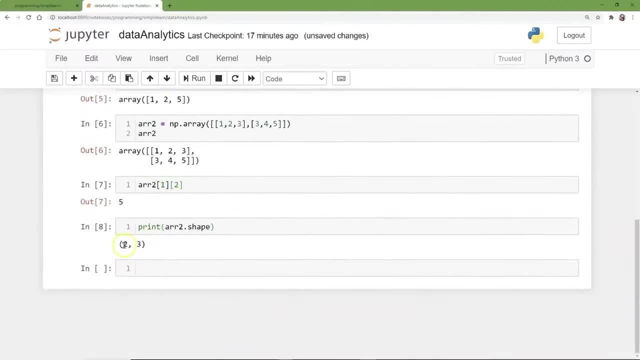 If you looked up here when we did it before, it just had 3, comma nothing. When you have a single entity, it always saves it as a tuple with a blank space. But you can see right here we have 2, comma 3.. 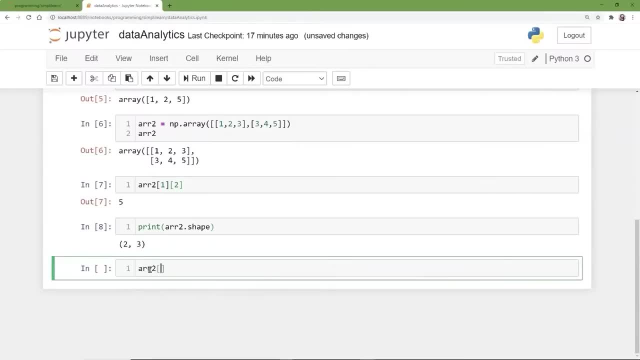 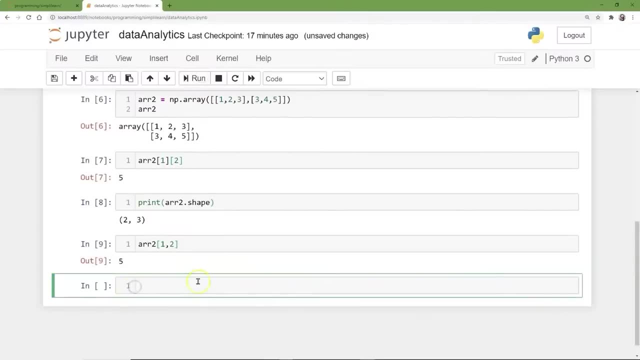 And if you remember from up here we just did this array2 of 1, comma 2.. We run that, We get the 5. We can also count backwards. This is kind of fun And you'll see, I just kind of switched something on you because you can also do 1, comma 2. 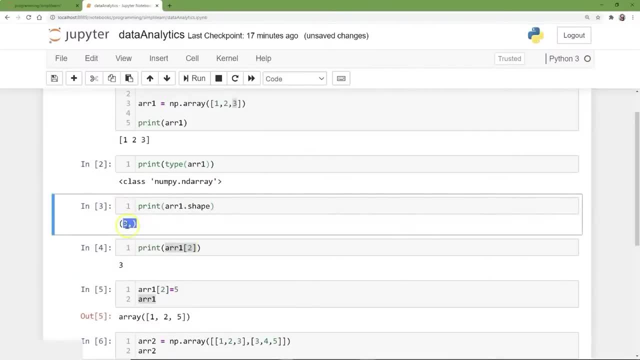 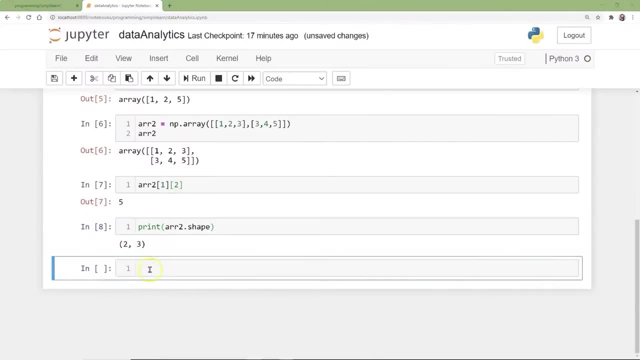 When you have a single entity it always saves it as a tuple with a blank space. But you can see, right here we have two comma three And if you remember from up here we just did this array two of let's go. what is it? 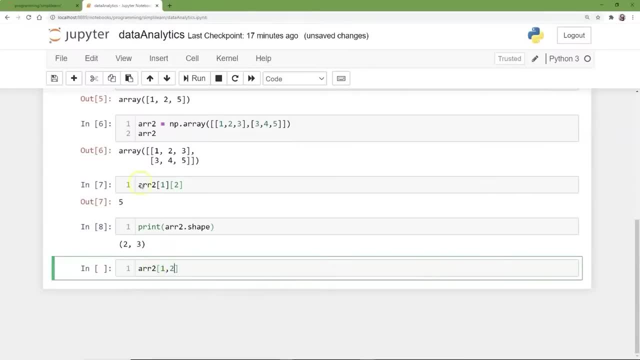 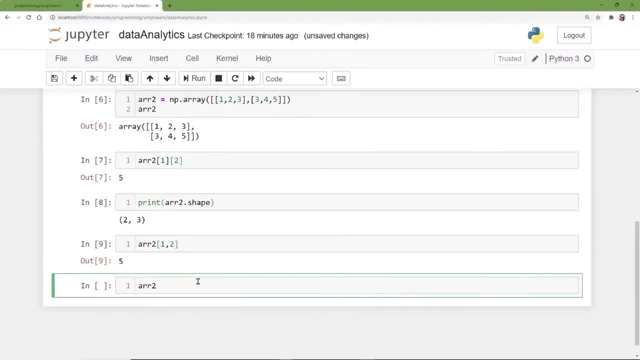 One comma two, We run that, We get the five. You can also count backwards. This is kind of fun And you'll see, I just kind of switched something on you because you can also do one comma two to get to the same spot. 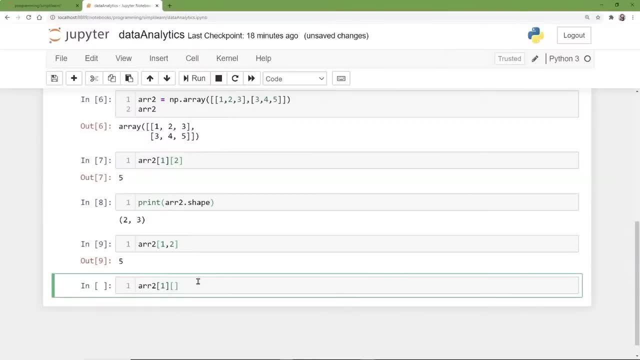 Now, two is the last one, Zero one. two: It's the last one in there. We can count backwards and do minus one, And if we run this we get the same answer, Whether we count it as. let's go back up here. 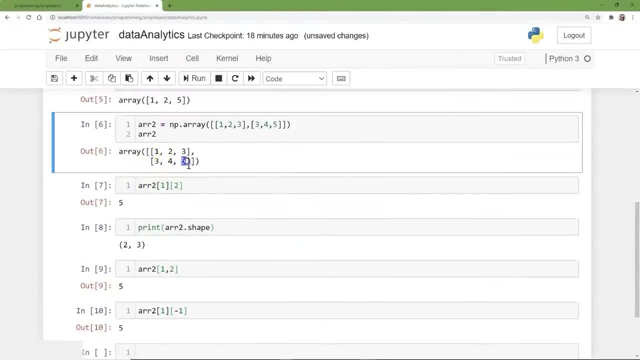 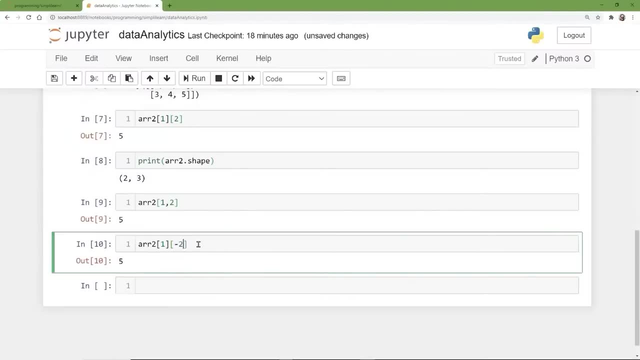 Whether we count this as zero, one, two or we count backwards as minus one, minus two, minus three, And you can see that if I change this minus one to a minus two and run that, I get four, which is going backwards. 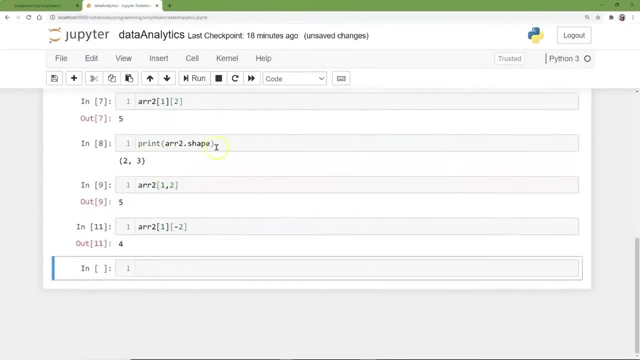 Minus one minus two, So there's a lot of different ways to reference what we're working on inside the numpy array. It's really a cool tool. It's got a lot of things you can do with it, And we talked about the fact. 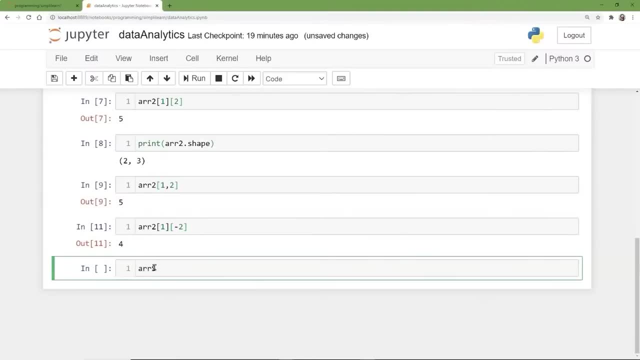 that it can also hold things that are not values, And we'll call this array. ask for strings equals nparray. Put our setup in there, brackets, And let's go: China, India, USA, Mexico, It doesn't matter, We can make whatever we want on here. 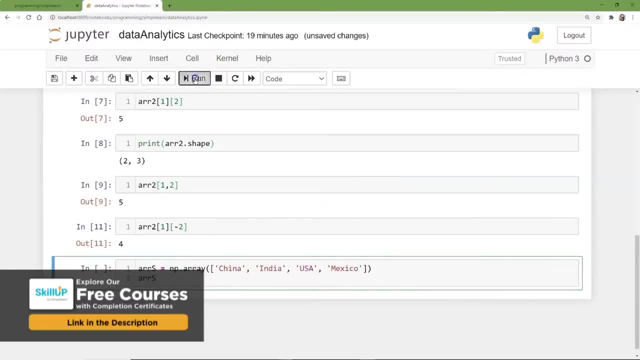 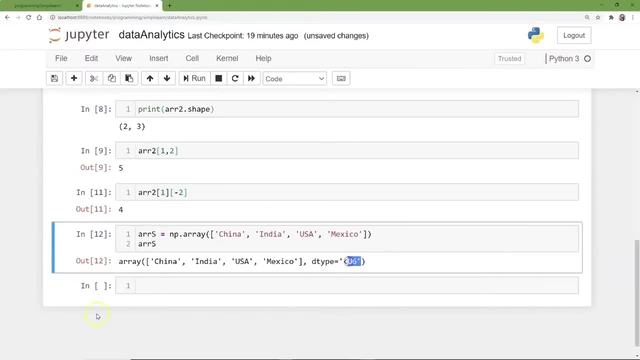 And if we print that out, we run this, you can see that we get our numpy array: China, India, USA, Mexico. It even gives us our dtype of a U6.. And a lot of times when you're messing with data. 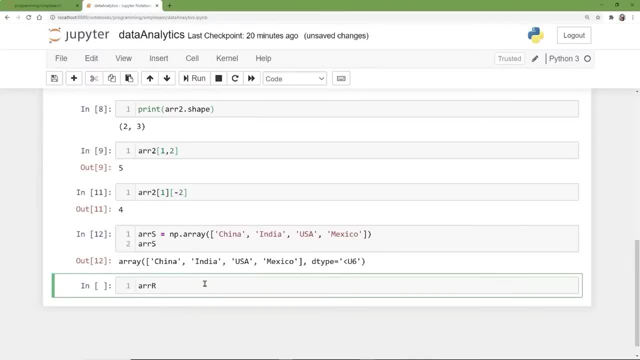 we'll call this array r for range, just to kind of keep it uniform- nparrange. So this is a command inside numpy to create a range of numbers, And if you're testing data, maybe you have equal time increments that are spaced a certain point apart. 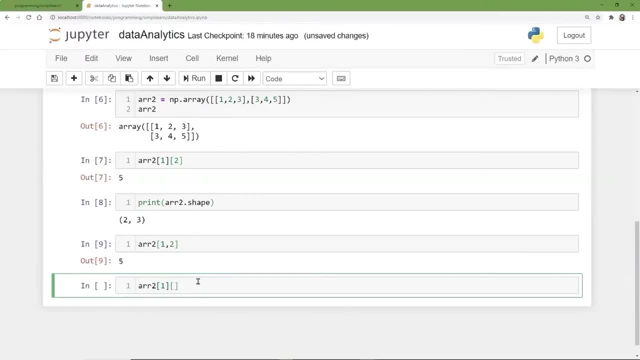 to get to the same spot. Now, 2 is the last, 1.. 0, 1, 2.. It's the last one in there. We can count backwards and do minus 1.. And if we run this, we get the same answer. 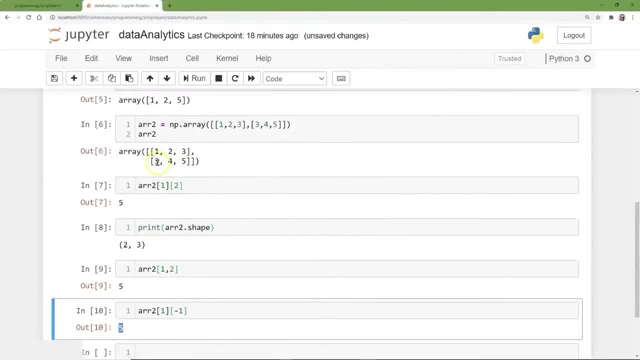 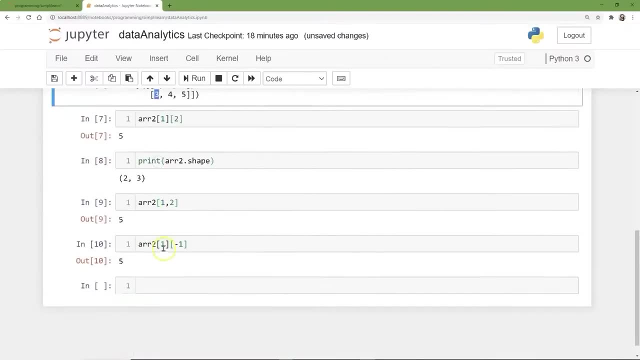 Whether we count it as- let's go back up here- Whether we count this as 0,, 1,, 2, or we count backwards as minus 1, minus 2,, minus 3.. And you can see that if I change this minus 1 to a minus 2 and run that, I get 4, which is going backwards. 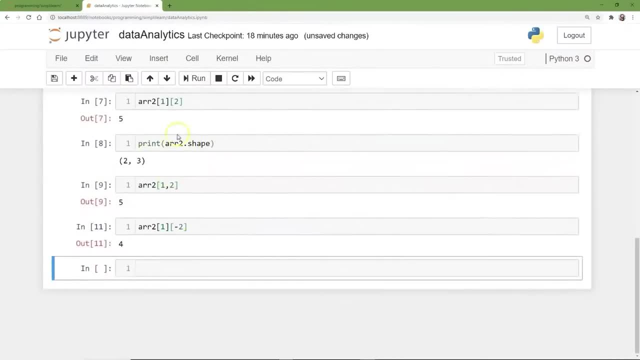 Minus 1, minus 2.. So there's a lot of different ways to reference what we're working on inside the numpy array. It's really a cool tool. It's got a lot of things you can do with it, And we talked about the fact that it can also hold things that are not values. 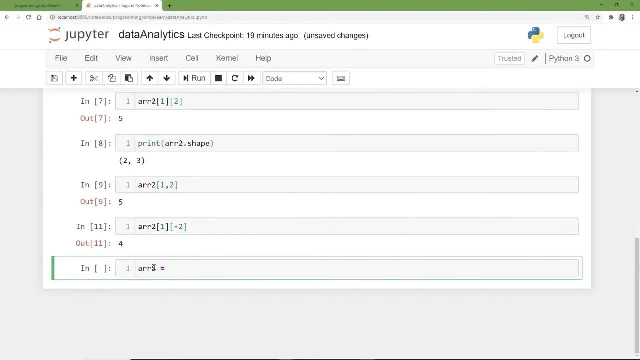 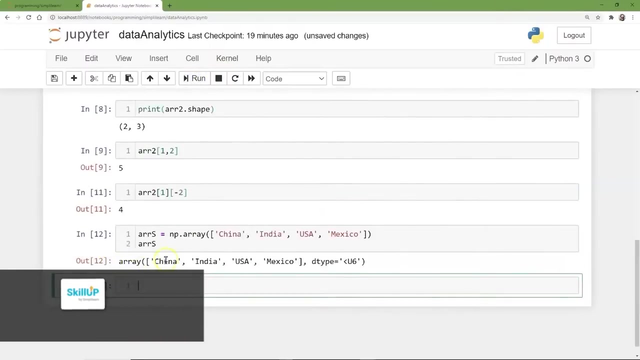 And we'll call this array s for strings equals nparray. Put our setup in there, brackets, And let's go: China, India, USA, Mexico, It doesn't matter, We can make whatever we want on here, And if we print that out, we run this, you can see that we get our numpy array: China, India, USA, Mexico. 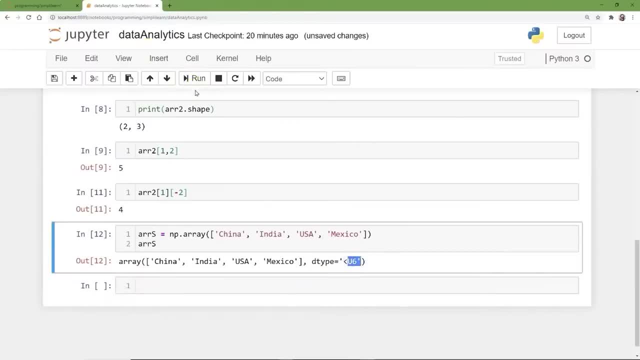 It even gives us our dtype of a user And we'll call this array r for range, just to kind of keep it uniform, nparange. So this is a command inside numpy to create a range of numbers, And if you're testing data, maybe you have equal time increments that are spaced a certain point apart. 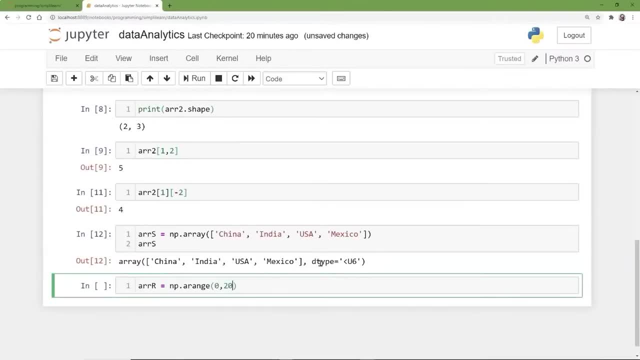 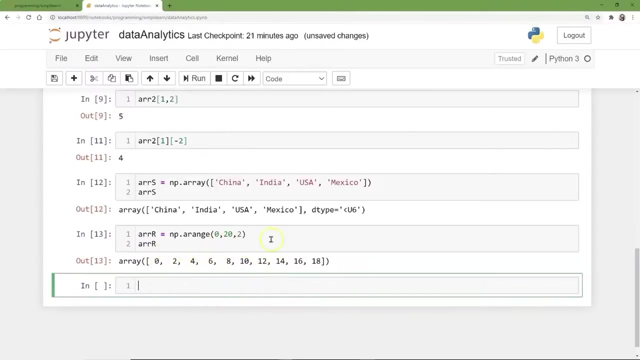 But in this case we're just going to do integers And we're going to do a setup from 0, 20, skipping every other one- And we'll print it out and see what that looks like. And you can see, here we have 0,, 2,, 4, 6, 8, 10,, 12,, 14,, 16,, 18.. 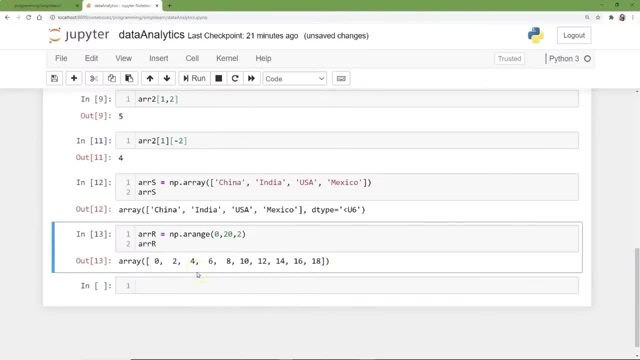 And, like you expected, it skips every one. And just a quick note: there's no 20 on here. Why, Well, this starts at 0 and counts up to 20.. And you're used to another language where it explicitly says less than or less than equal to 20,. 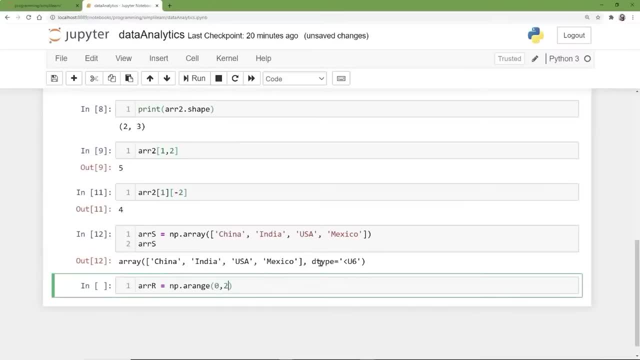 But in this case we're just going to do integers And we're going to do a setup from 0, 20, skipping every other one- And we'll print it out and see what that looks like And you can see here. 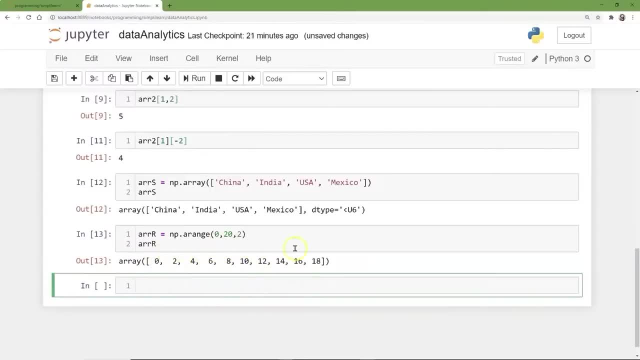 we have 0,, 2,, 4,, 6,, 8,, 10,, 12,, 14,, 16,, 17,, 18,. like you expected, It skips every one. And just a quick note, there's no 20 on here. 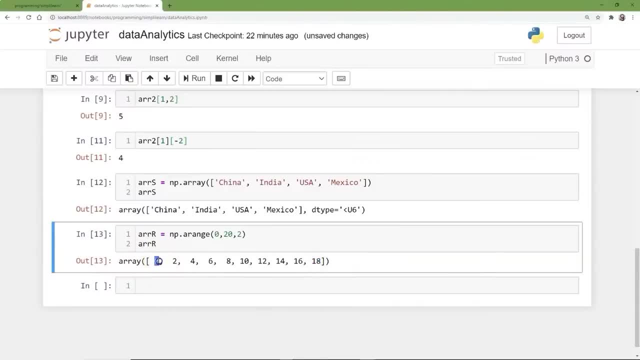 Why? Well, this starts at 0 and counts up to 20.. So if you're used to another language where it explicitly says less than or less than equal to 20, like for, x equals 0,, x plus plus x is less than 20.. 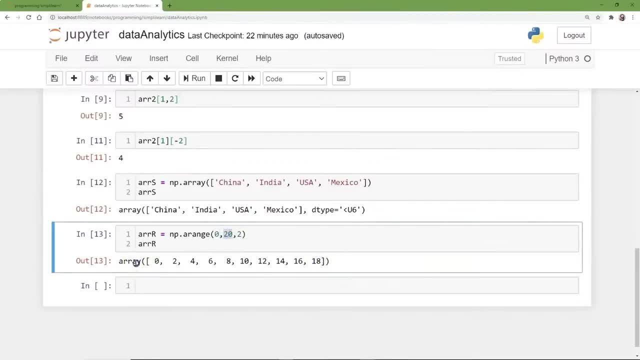 That's what this is. It just assumes x is less than 20 on here. And if we want to create a very uniform set- you know 0,, 2,, 4, 6, what happens if I want to create numbers? 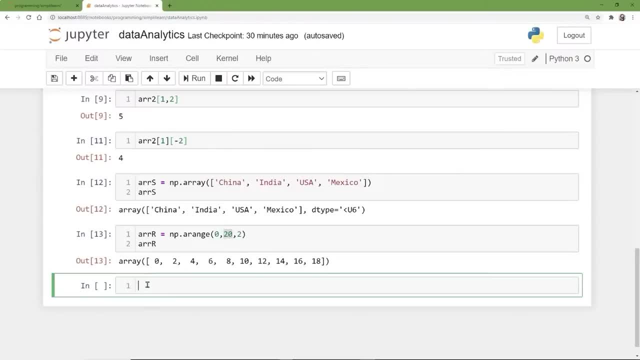 from 0 to 10, but I need 20 increments in there. We can do that with line space, So we can create an r. We'll call this l equals. I don't think we'll actually use any of this again. 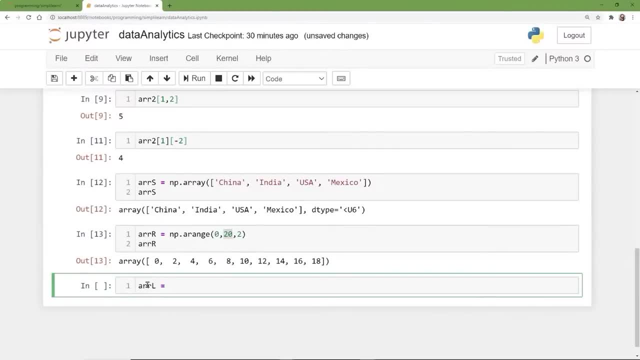 so I don't know why I'm creating unique identifiers for it. But we'll do np lin space and we're going to do 0 to 10, or 0 to 9.. Remember, it goes up to 10.. 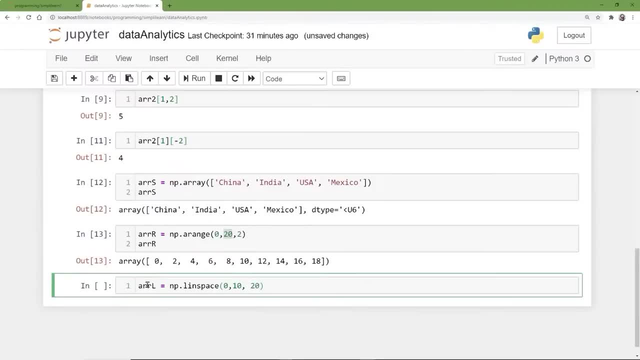 And then we want to. let's say, we have 20 different increments in there. So we have a data set and we know it's over a certain time period and we need to divide that time period by 20.. And it happens to just have 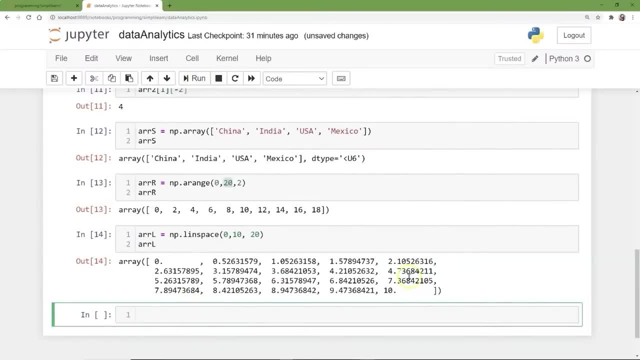 10 pieces in it. And here we go. You can see, right here we have 20, or it has 20 pieces in it, but it's over 10 years. We've got to divide it in the middle And you can see it does. 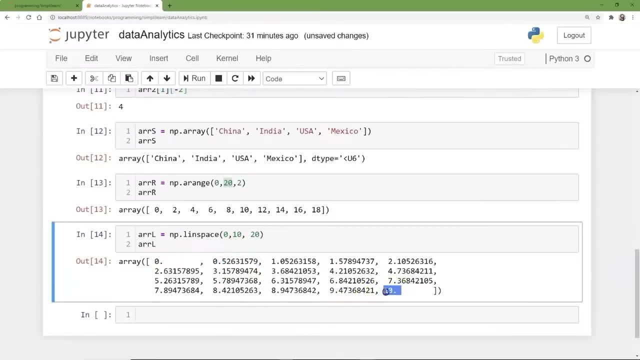 it goes 0.52.. Remember, yeah, there's our 10 on the end, so it goes up to 10.. And then we can also do random. There's nprandom. If you're doing neural networks, usually you start it by. 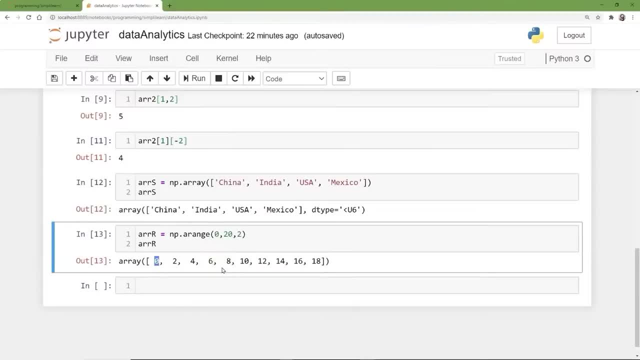 like for, x equals 0, x plus plus x is less than 20.. That's what this is. It just assumes x is less than 20 on here. And if we want to create a very uniform set- 0,, 2,, 4,, 6,. 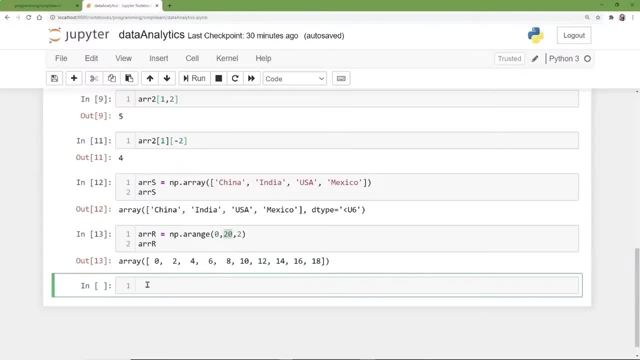 what happens if I want to create numbers from 0 to 10, but I need 20 increments in there? Well, we can do that with line space, So we can create an r. We'll call this: l equals. I don't think we'll actually use any of this again. 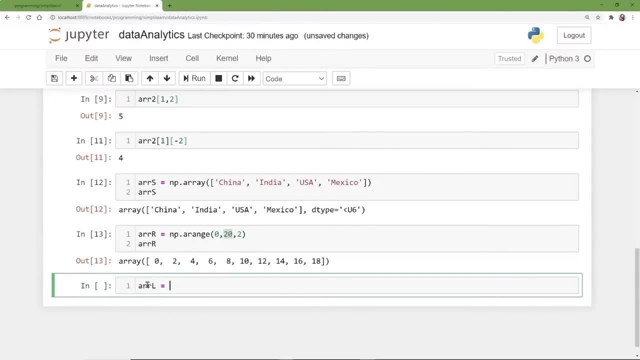 so I don't know why I'm creating unique identifiers for it. But we'll do np lin space And we're going to do 0 to 10, or 0 to 9.. Remember, it goes up to 10. And then we want to- let's say we have 20.. 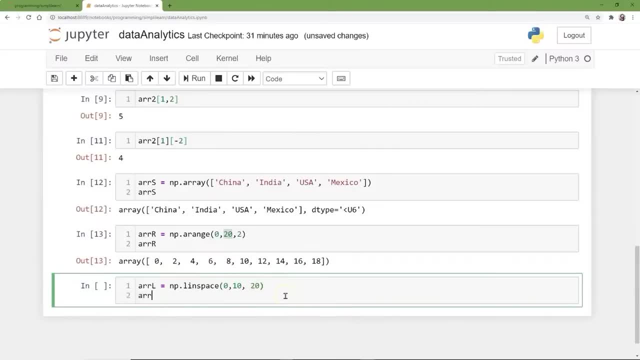 So we're going to put in different increments in there. So we have a data set and we know it's over a certain time period And we need to divide that time period by 20. And it happens to just have 10 pieces in it. 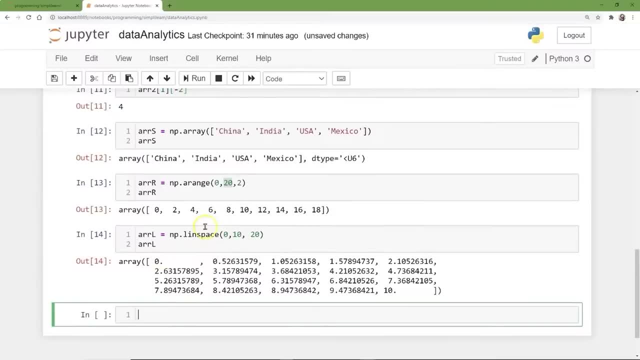 And here we go. You can see right here, it has 20 pieces in it, but it's over 10 years And we've got to divide it in the middle And you can see it goes 0.52.. Remember, yeah, there's our 10 on the end, so it goes up to 10.. 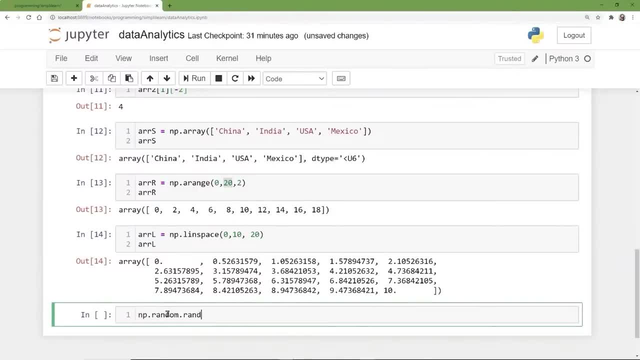 And then we can also do random nprandom. If you're doing neural networks, usually you start it by seeding it with random numbers And we'll just do nprandom And we'll just call this array, We'll stop giving it unique numbers. 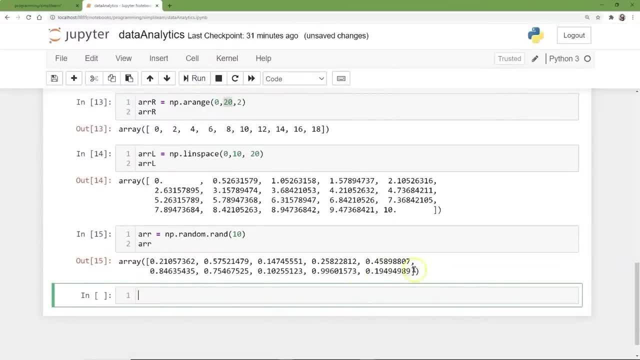 We'll print that one out and run it And you can see we have random numbers. They are 0 to 1.. So you'll see that all of these numbers are under 1. And you can easily alter that by multiplying them out or something like that. 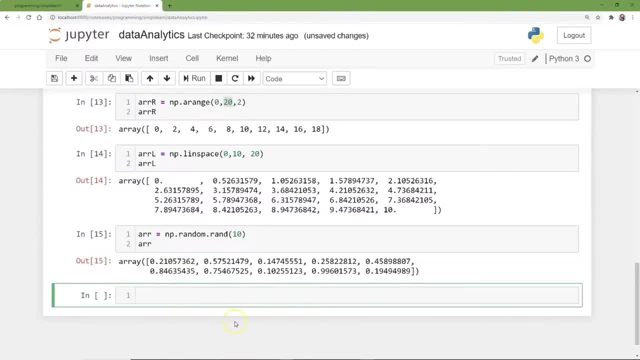 if you want to do like 0 to 100. You can also round them up if it's integers 0 to 100. There's all kinds of things you can do, But it generates a random float between 0 and 1.. 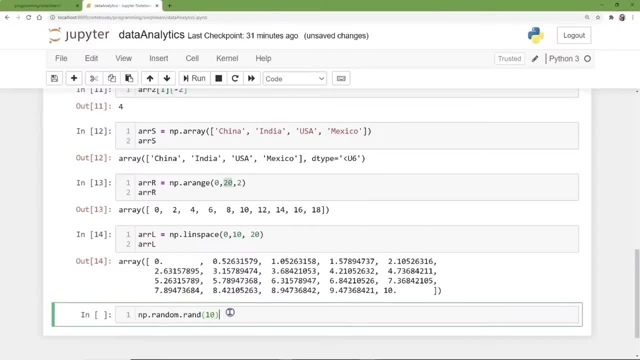 seeding it with random numbers And we'll just do nprandom and we'll just call this array, We'll stop giving it unique numbers. We'll print that one out and run it And you can see we have random numbers. They are 0 to 1.. 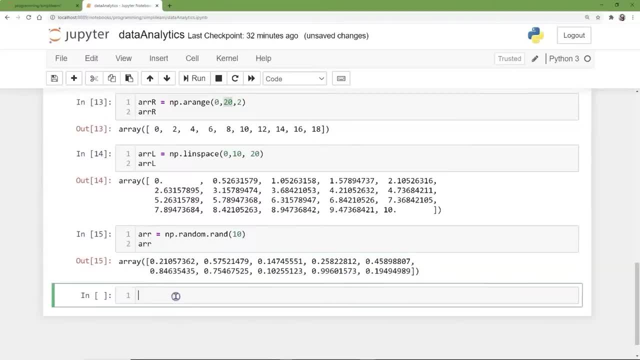 So you'll see that all these numbers are under 1. And you can easily alter that by multiplying them out or something like that if you want to do like 0 to 100.. You can also round them up if it's integer 0 to 100.. 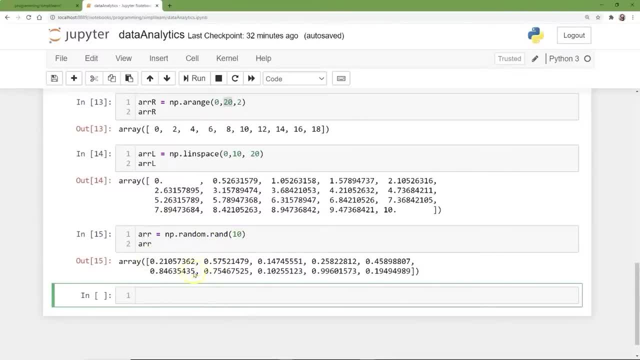 There's all kinds of things you can do, but it generates a random float between 0 and 1.. And you have a couple options. You could reshape that, or you can just generate them in whatever shape you want, And so we can see here. 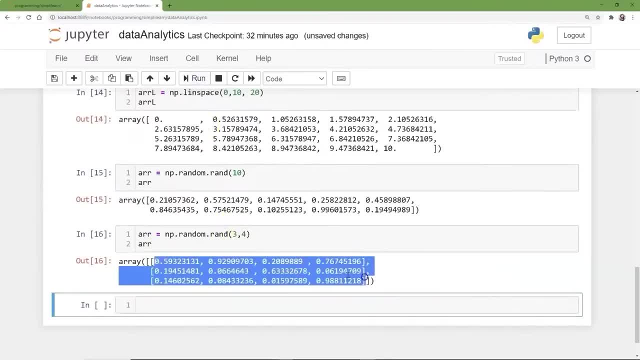 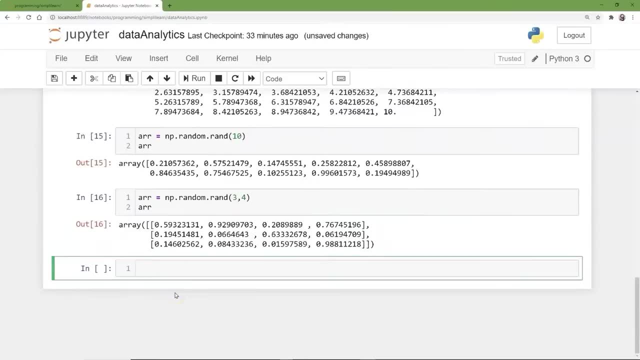 we did 3 and 4. And so you can see 3 rows by 4 variables. Same thing as doing a reshape of 12 variables to 3 and 4. And if you're going to do that, you might need an empty data set. 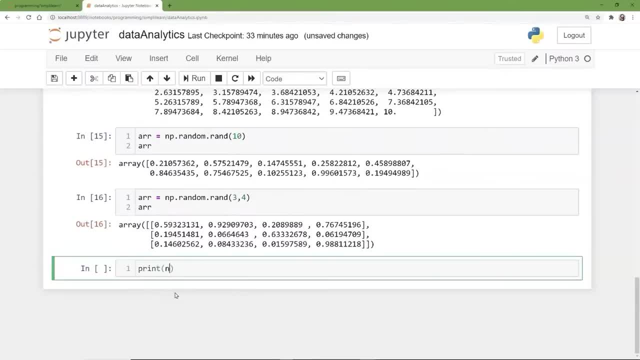 I have had this come up many times. Or I need to start off with 0. And I don't know, you know, because I'm going to be adding stuff in there, Or it might be 0 and 1, but the reason is, if you're 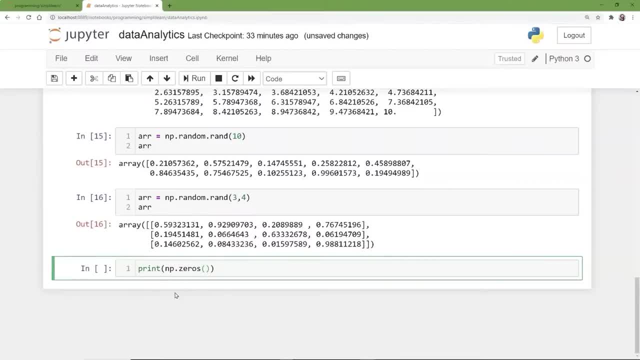 removing the background of an image you might want. the background is 0. And then you figure out where the image is and you set all those boxes to 1, and you create a mask. So creating masks over images is really big. 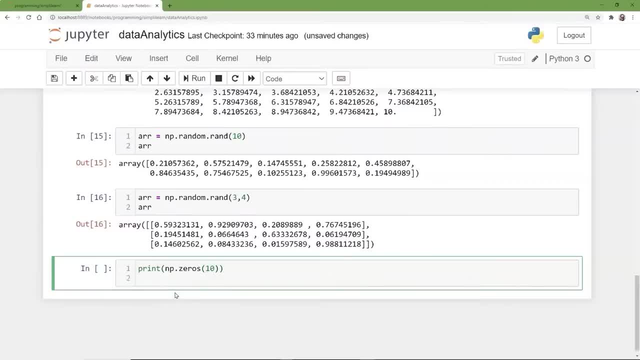 and doing that with a numpy array of 0. And we can also give it a space, And we'll just do this all in one shot this time, And we'll do the same thing like we did before: 0s, and in this case, 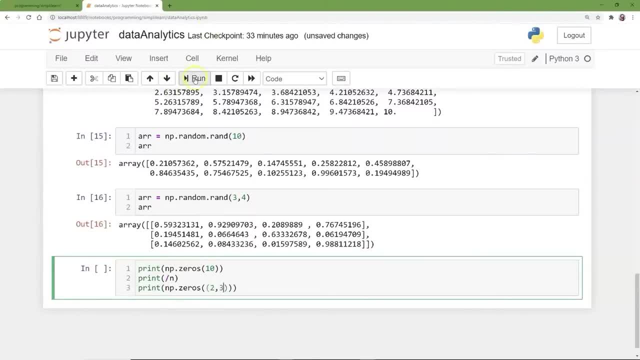 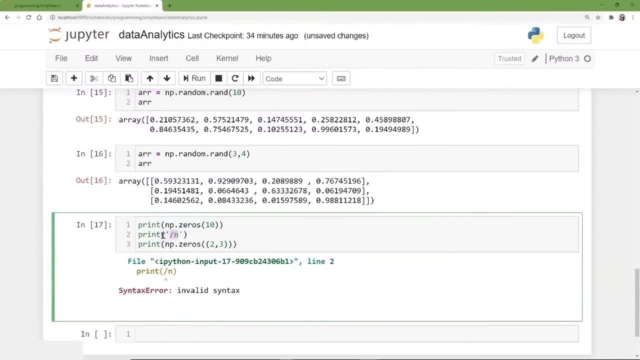 we'll do 2,, 3.. And so when we run this, I forgot the asterisks around it. I knew I was forgetting something. There we go. So when we run this, you can see, here we have our 10 0s in a row. 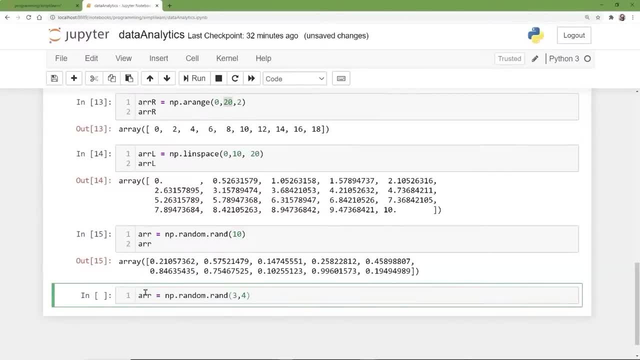 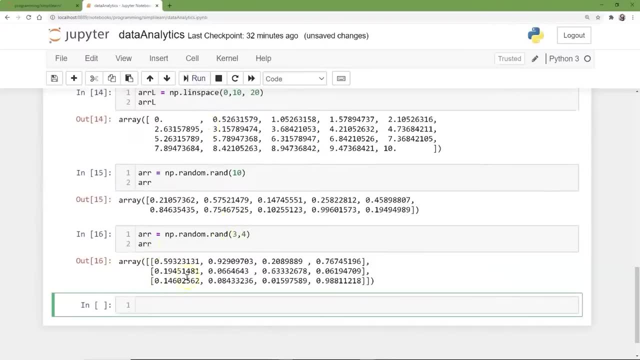 And you have a couple options. You could reshape that, Or you can just generate them in whatever shape you want, And so we can see here we did 3 and 4.. And so you can see 3 rows by 4 variables. 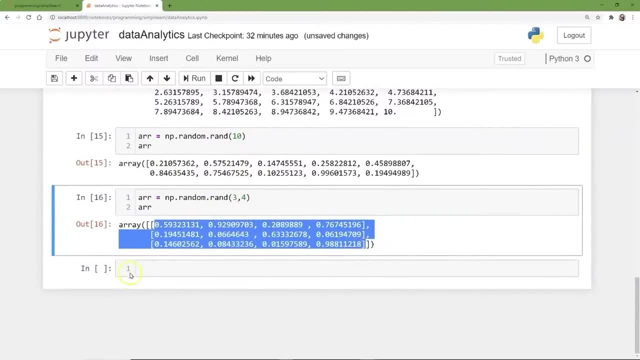 Same thing as doing a reshape of 12 variables to 3 and 4.. And if you're going to do that, you might need an empty data set. I have had this come up many times, Or I need to start off with 0.. 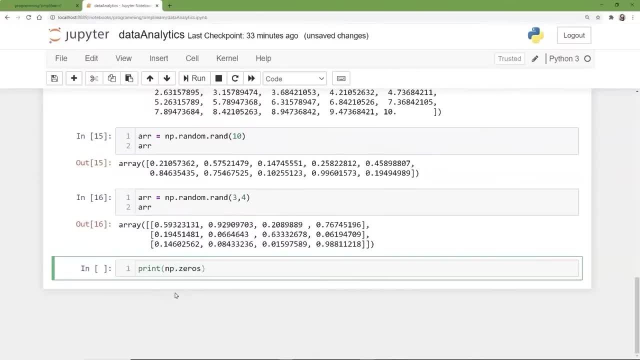 And I don't know. you know, because I'm going to be adding stuff in there- Or it might be 0 and 1.. Or 1 is if you're removing the background of an image you might want. the background is 0.. 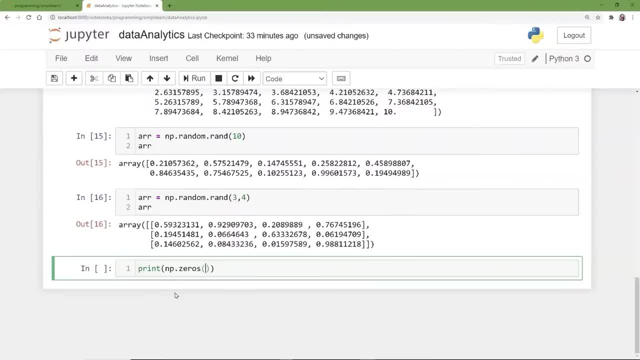 And then you figure out where the image is And you set all those boxes to 1. And you create a mask. So creating masks over images is really big, And doing that with a numpy array, An array of 0. And we can also give it a space. 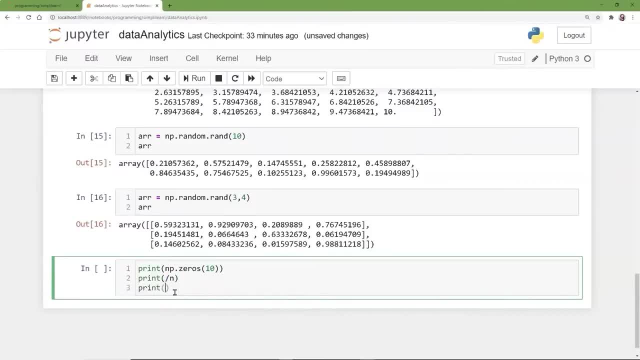 And we'll just do this all in one shot this time, And we'll do the same thing like we did before: Zeros, And in this case we'll do 2 comma 3.. And so when we run this, I forgot the asterisk around it. 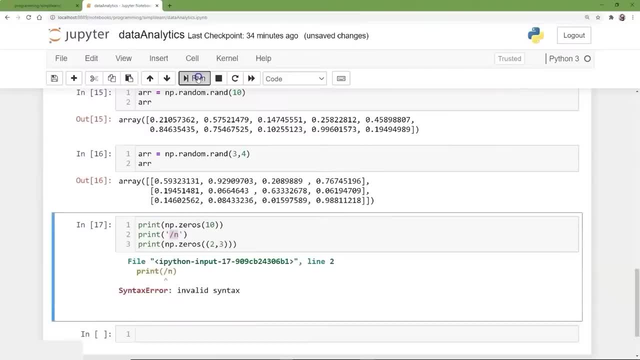 I knew I was forgetting something. There we go. So when we run this, we can see: here we have our 10 zeros in a row- And maybe this is a mask for an image- And so it has 2 rows of 3 digits in it. 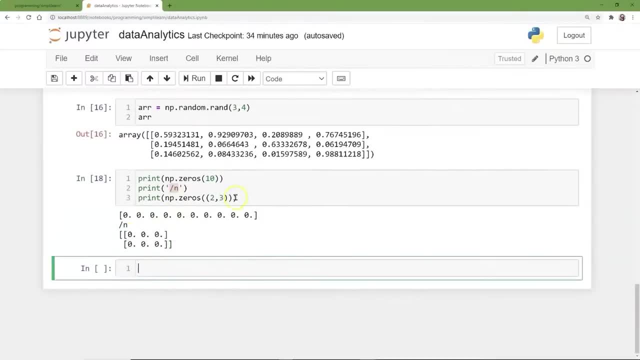 So it's a very small image, A little tiny pixel, And maybe you're looking to do something the opposite way. Instead of creating a mask of 0s and filling in with 1s, Maybe you want to create a mask of 1s. 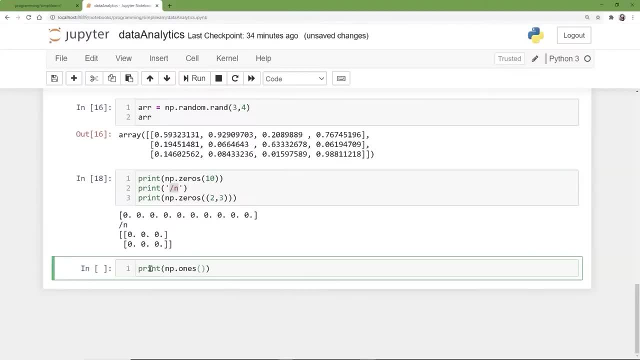 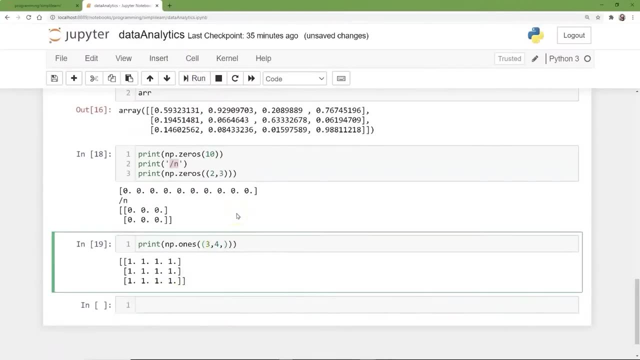 And fill them in with 0s, And we'll just do Just like we did before. We'll do 3 comma 4.. And when we run this you'll see it's all 1s And we can even do this even. 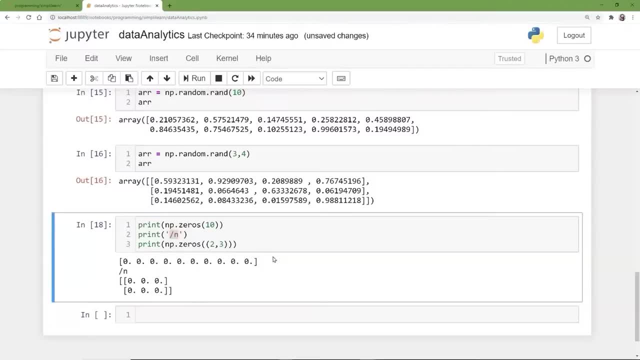 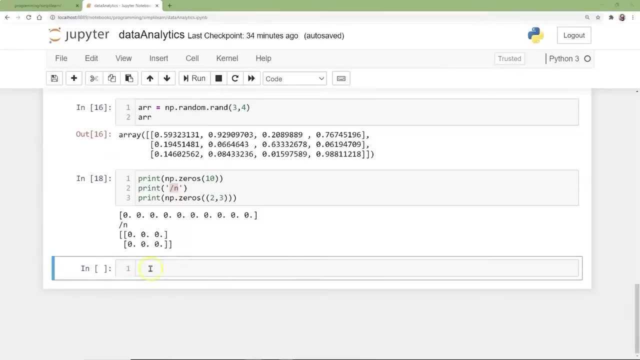 And maybe this is a mask for an image, And so it has 2 rows of 3 digits in it. So it's a very small image, a little tiny pixel, And maybe you're looking to do something the opposite way, Instead of creating a mask of 0s. 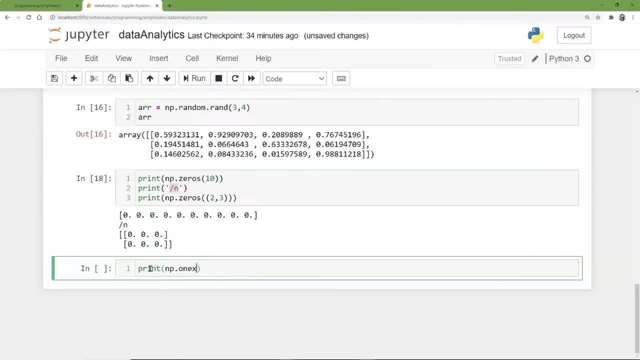 and filling in with 1s. maybe you want to create a mask of 1s and fill them in with 0s, And we'll just do just like we did before. we'll do 3,, 4. And when we run this, 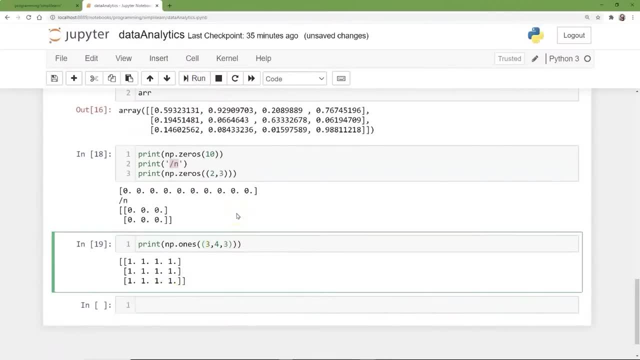 you'll see it's all 1s And we can even do this. even we'll do it this way: Let's do 10, 10 by 10 icon and then you have your 3 colors. So it creates quite a large array there. 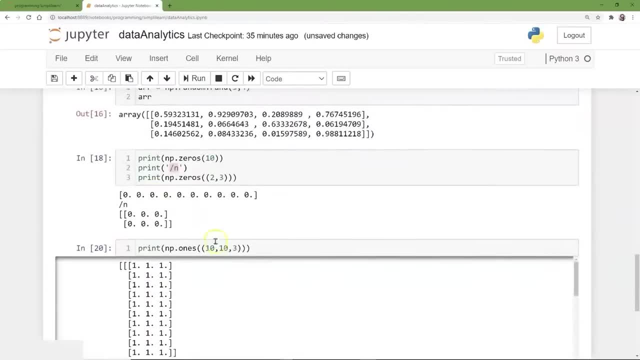 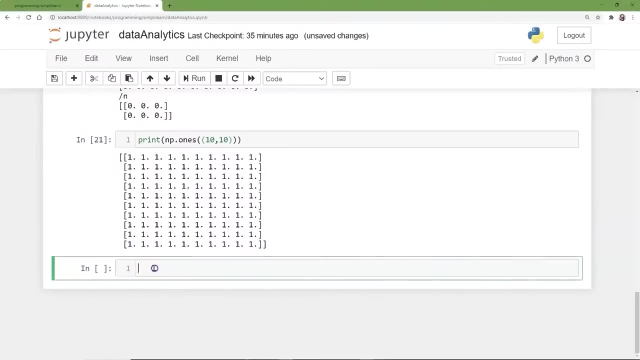 for doing pictures and stuff like that. when you add that third dimension in, If we take that off, it's a little bit easier to see. We'll do 10 again And you can easily see how we have 10 rows of 10 1s. 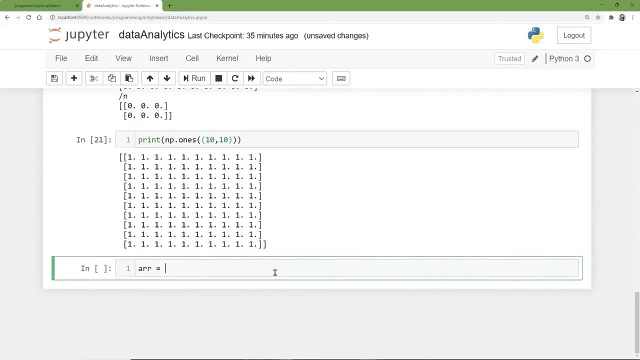 And you can also do something like create an array And we'll do 0,, 1,, 2.. And then in this array we actually print right out: we want a repeat, So you can actually do a repeat of the array. 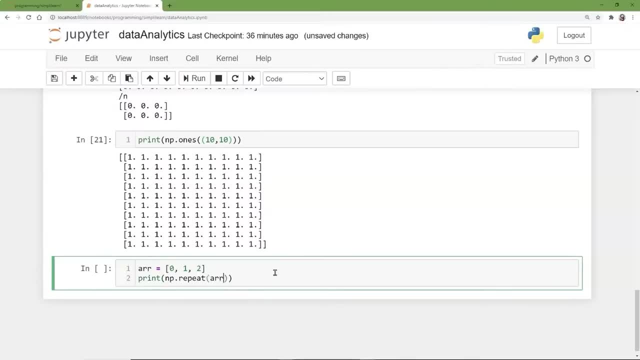 and maybe you need this array. let's repeat it 3 times. So there's our repeat of an array. repeat 3 times And if we run this, you'll see we have 0, 0, 0, 1, 1, 1, 2, 2, 2.. 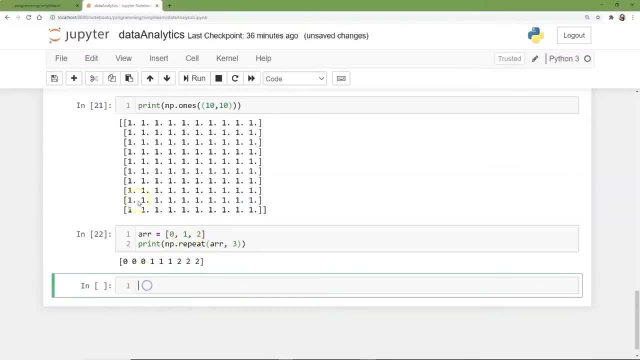 And whenever I think of a repeat, I don't really think of repeating being the first digit 3 times the second digit. I really always think of it as 0, 1, 2, 0, 1, 2, 0, 1, 2.. 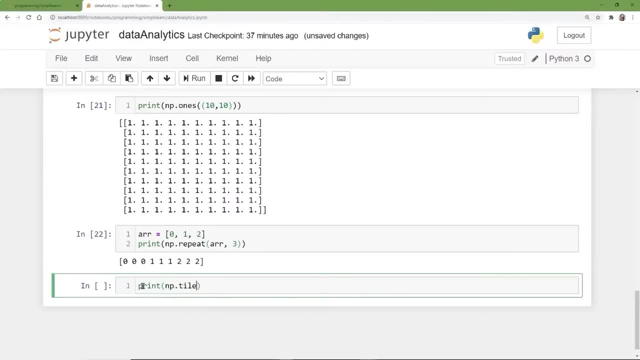 It catches me every time, But the actual code for that one is going to be tile. And again, if we do arrange 3, and we run this, you can see how you can generate 0, 1, 2, 0, 1, 2, 0, 1, 2.. 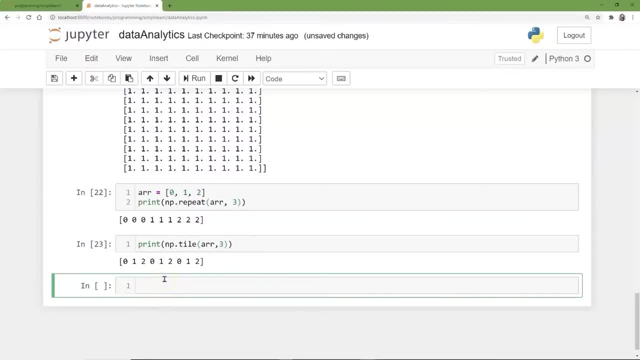 And if you're dealing with an identity matrix, we can do that also. if you're big on, you're doing your matrixes And we'll just identity. I guess we'll go ahead and spell it out today: Matrix And the command we're looking for. 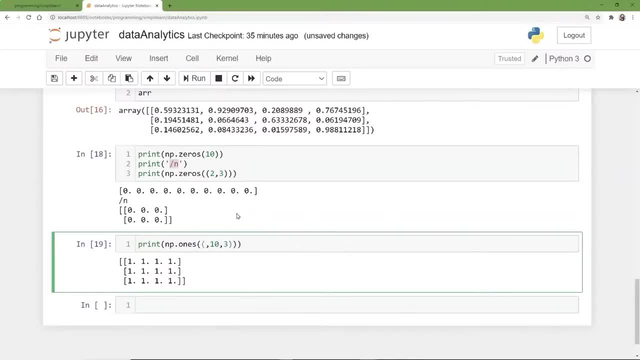 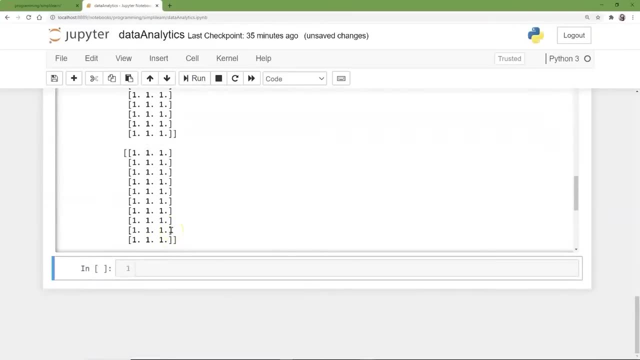 We'll do it this way. Let's do 10.. 10 by 10 icon And then you have your 3 colors. So it creates quite a large array there for doing pictures and stuff like that, When you add that third dimension in. 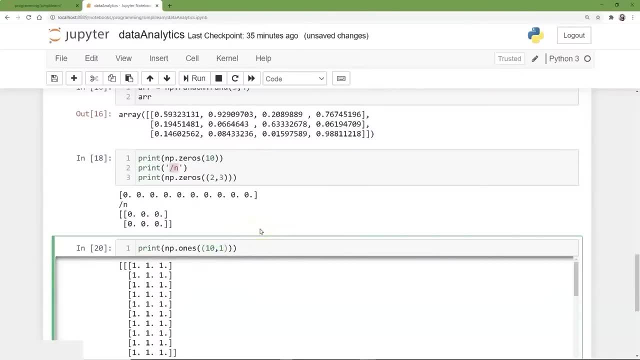 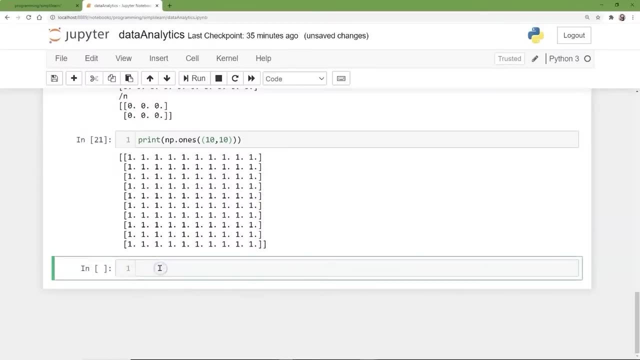 If we take that off, it's a little bit easier to see. We'll do 10 again And you can easily see how we have 10 rows of 10 1s. And you can also do something like create an array And we'll do 0, 1, 2.. 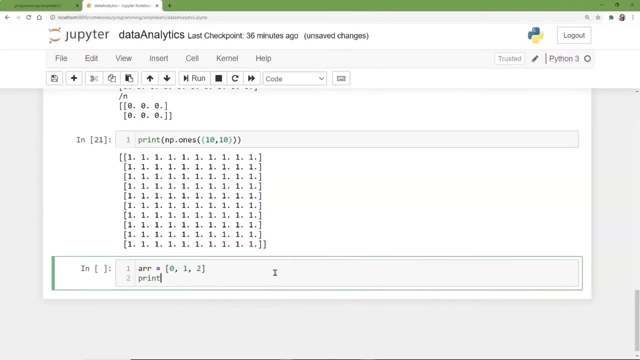 And then in this array We actually Print right out: We want a repeat So you can actually do a repeat of the array And maybe you need this array. Let's repeat it 3 times. So there's our repeat of an array. 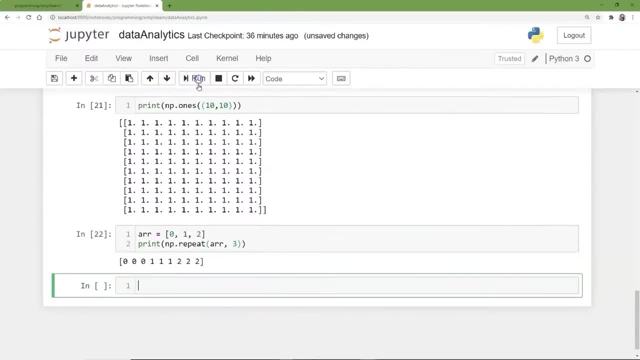 Repeat 3 times And if we run this, You'll see we have 0, 0,, 0,, 1, 1, 1,, 2,, 2,, 2.. And whenever I think of a repeat, 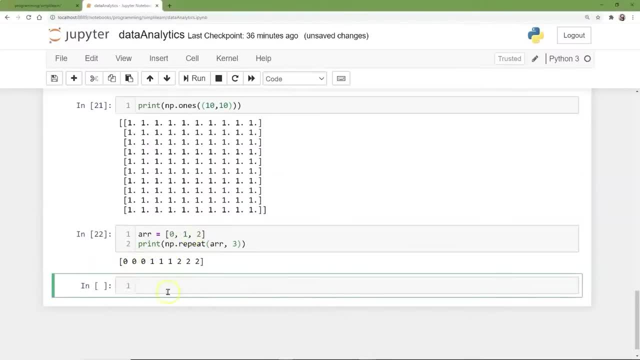 I don't really think of repeating being the first digit 3 times the second digit. I really always think of it as 0, 1, 2, 0, 1, 2, 0, 1, 2.. 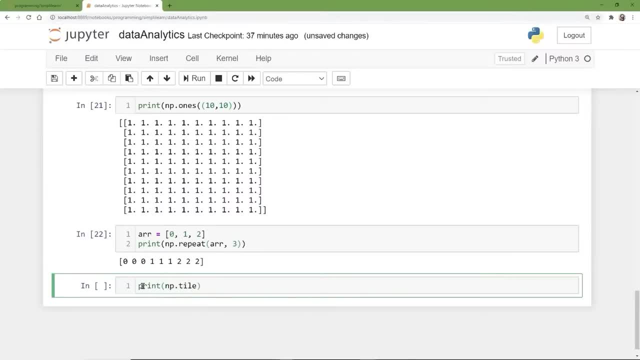 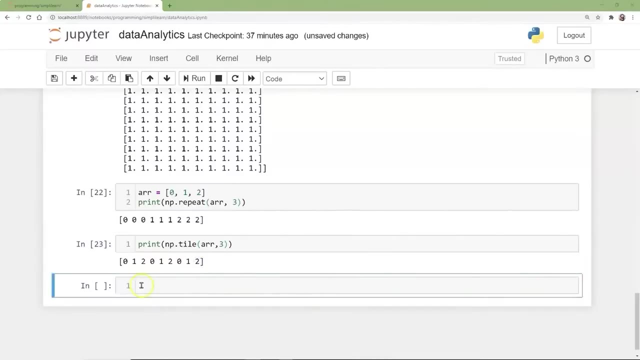 It catches me every time, But the actual code for that one Is going to be tile. And again, if we do arrange, 3.. And we run this. You can see how you can generate 0, 1, 2, 0, 1, 2, 0, 1, 2.. 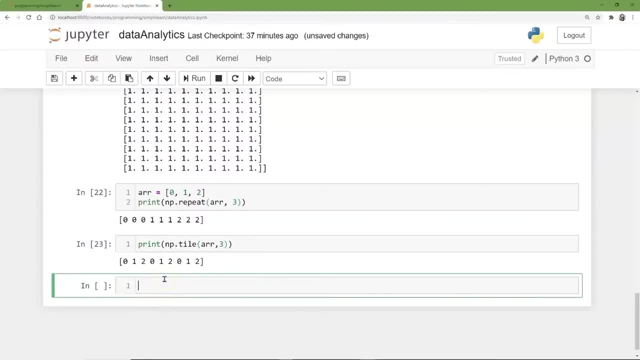 And if you're dealing with an identity matrix, We can do that also. if you're big on, you're doing your matrixes And we'll just identity. I guess we'll go ahead and spell it out today, Matrix And the command we're looking for is I. 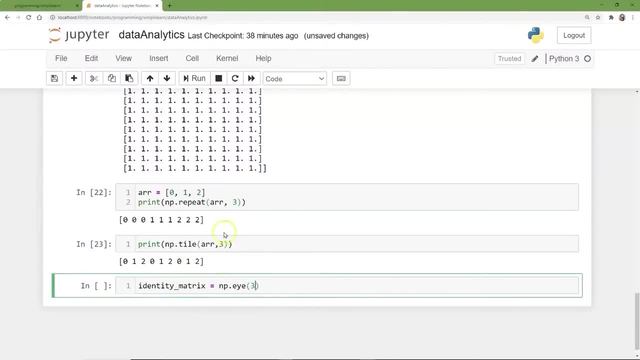 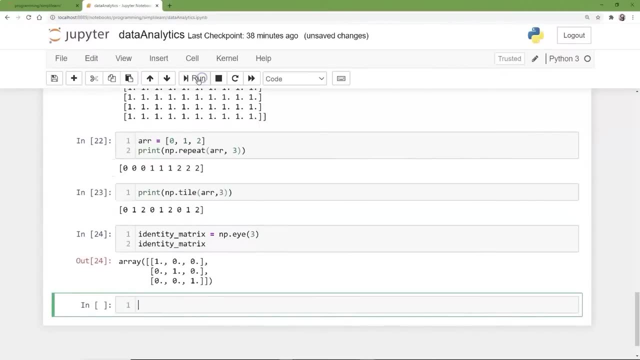 E-Y-E And we'll do 3.. And then we'll just go ahead and print this out. There we go, There's our identity matrix And it comes out by a 3 by 3 array, Because there's our matrix. 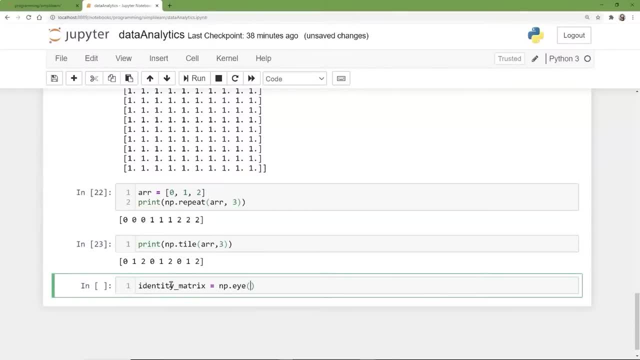 is I E-Y-E And we'll do 3.. And then we'll just go ahead and print this out. And then we'll just go ahead and print this out. There we go, There's our identity matrix, And it comes out by a 3 by 3 array. 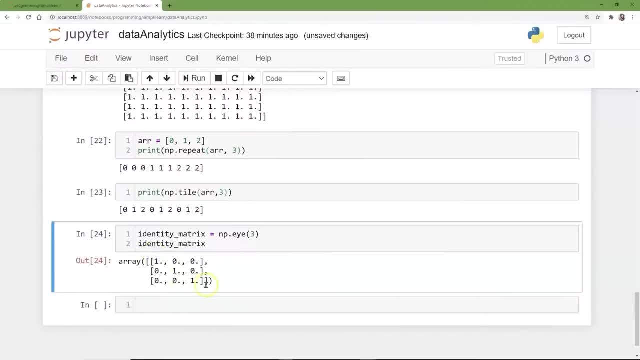 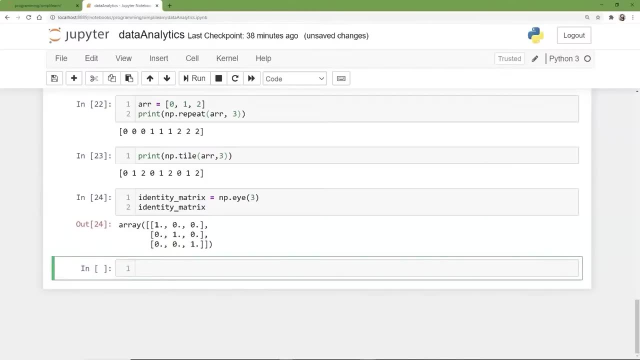 because there's our matrix And then it puts the ones down the middle for doing your different matrix math, And we can manipulate that a little bit too. When we talk about matrixes, we might not want ones across the middle, In which case 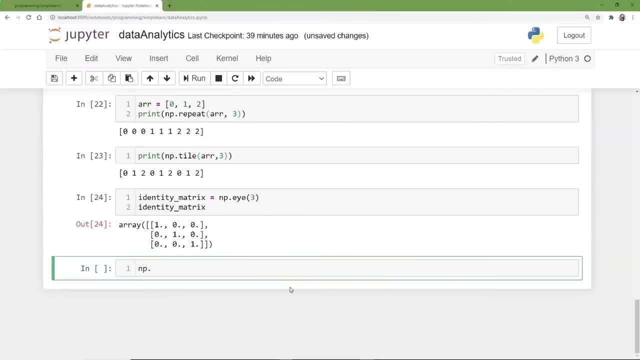 we now have the diagonal, So we can do an npdiagonal And we do a diagonal. Let's put in the diagonal 1,, 2,, 3,, 4,, 5. And when we run this again, this generates a value. 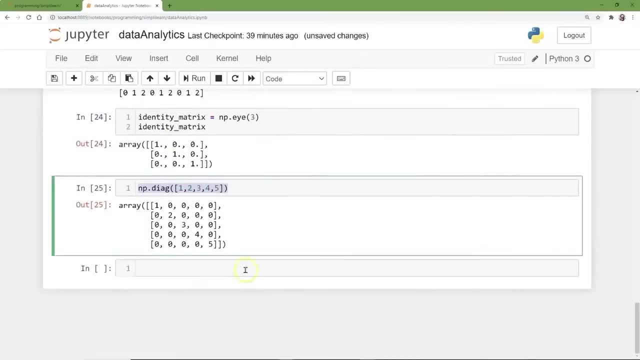 And by just putting that value in there's the same as putting print around it, Or putting array equals and then print array And you can see it generates a diagonal 1,, 2,, 3,, 4,, 5.. And there's your beginning. 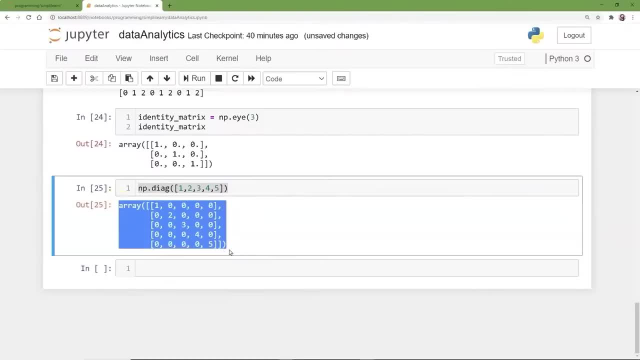 of your matrix array for working with matrixes. And we can actually go in reverse. Let's create an array equals- remember our random Randomrandom- And we'll do a 5 by 5 array. Oops, there we go, 5 by 5.. 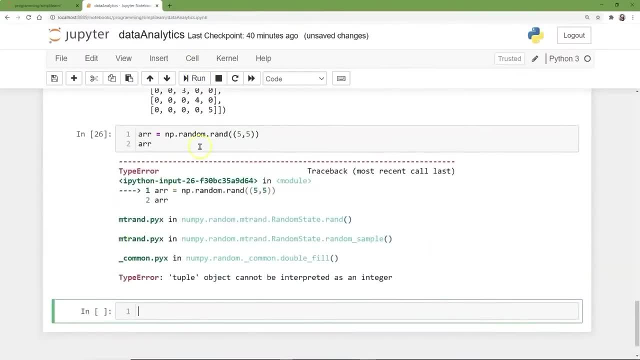 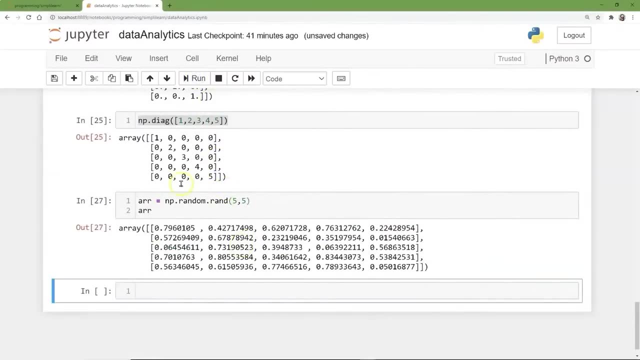 Just so you can see what that looks like Helps if I don't mistype the numbers, Which in this case, I just need to take out the brackets And there you go. You have your 5 by 5 array set up in there. 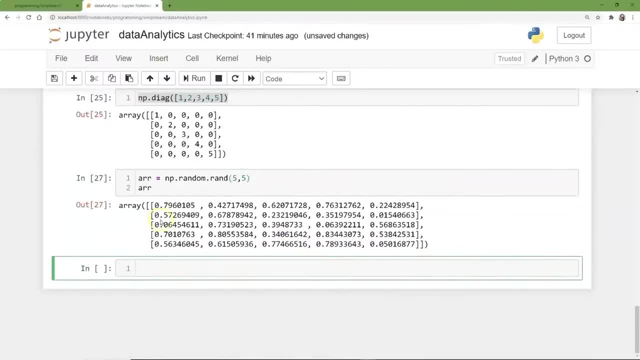 And we can now because we're working with matrixes. we might want to do this in reverse and extract the diagonals, Which would be the .79,, the .678 and so on, And we simply type in npdiagonal, We put our array in there. 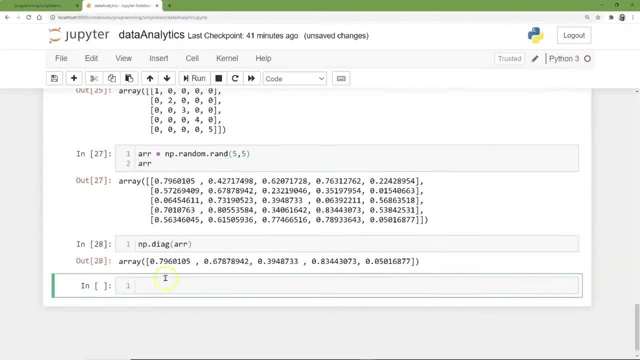 And this will, of course, print it out because it returns it as a variable And you can see here, here's our diagonal going across from our matrix, And we did talk about shape earlier. If you remember, you can do print the shape out. 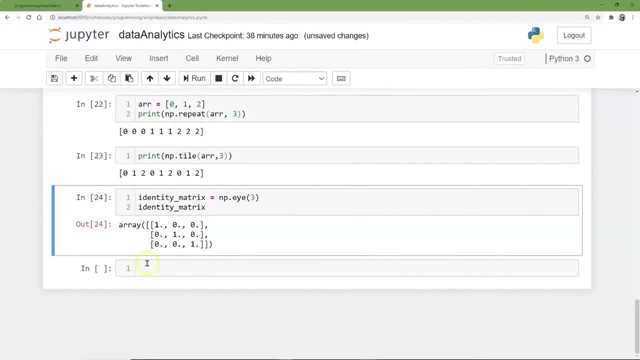 And then it puts the ones down the middle For doing your different matrix math, And we can manipulate that a little bit too. When we talk about matrixes, We might not want ones across the middle, In which case we now have the diagonal. 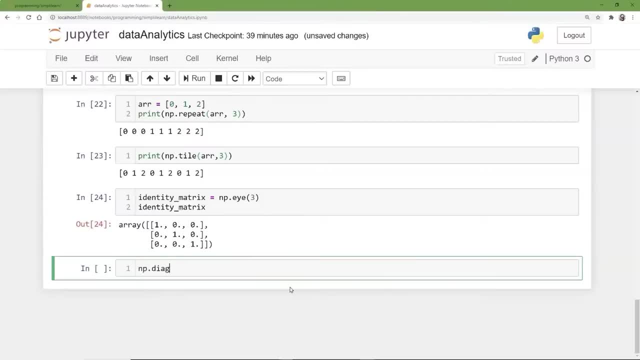 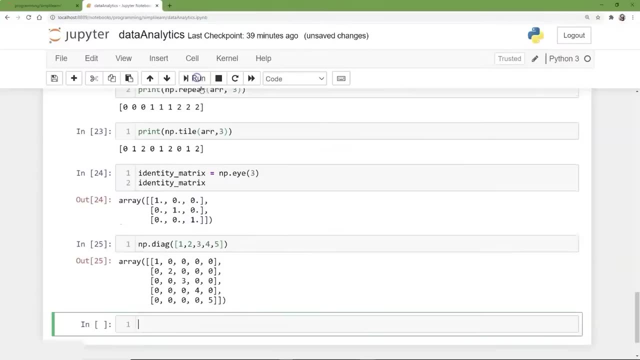 So we can do an npdiagonal And we do a diagonal. Let's put in the diagonal 1,, 2,, 3,, 4,, 5. And when we run this Again, this generates a value, And by just putting that value in, 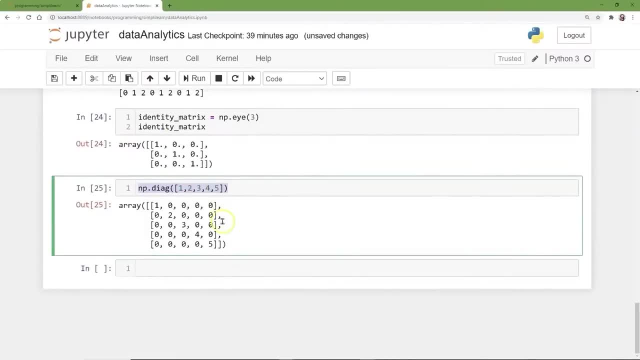 There's the same as putting print around it, Or putting array equals And then print array And you can see it generates a diagonal 1,, 2,, 3,, 4,, 5.. And there's your beginning of your matrix array. 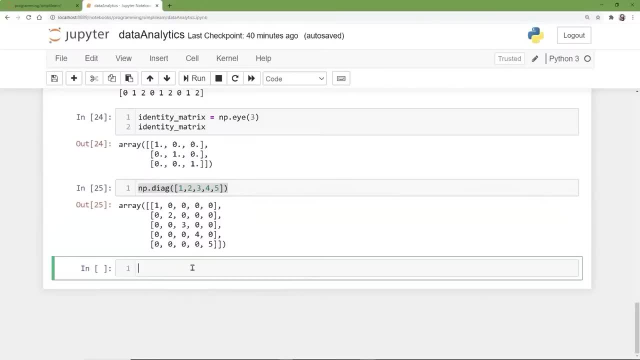 For working with matrixes, And we can actually go in reverse. Let's create an array Equals- Remember our random Randomrandom- And we'll do a 5 by 5 array. Oops, There we go, 5 by 5.. 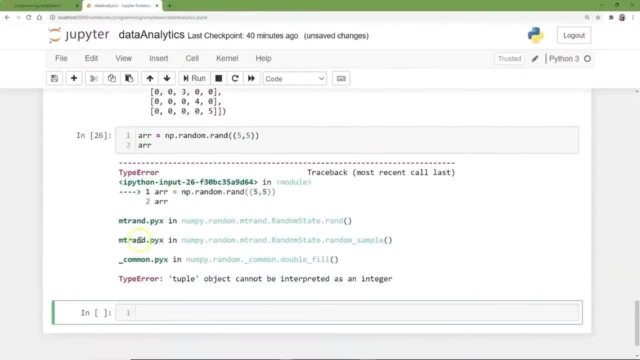 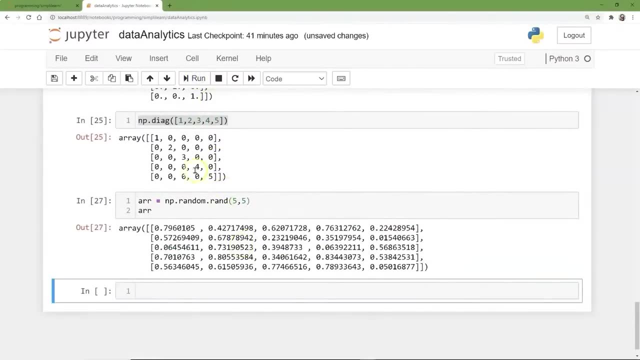 Just so you can see what that looks like Helps if I don't mistype the numbers, Which in this case, I just need to take out the brackets And there you go. You have your 5 by 5 array set up in there. 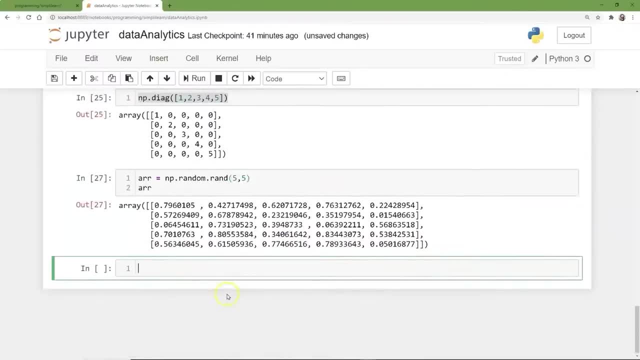 And we can now, Because we're working with matrixes. We might want to do this in reverse And extract the diagonals, Which would be the .79.. The .678. And so on, And we simply type in npdiagonal. 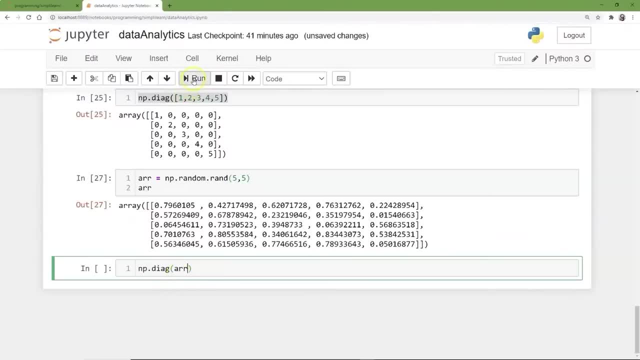 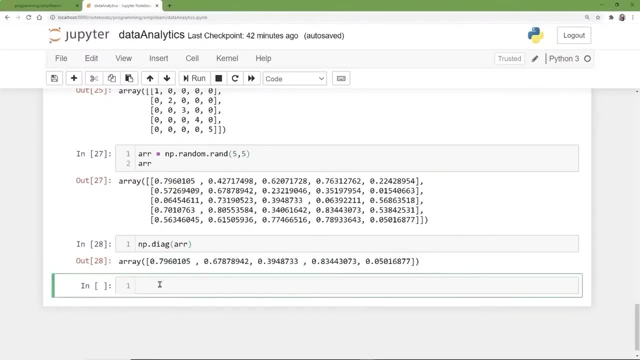 We put our array in there And this will, of course, print it out Because it returns it as a variable And you can see here. Here's our diagonal going across from our matrix, And we did talk about shape earlier, If you remember. you can do. 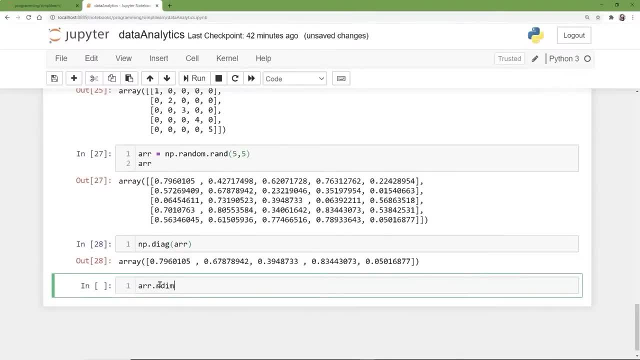 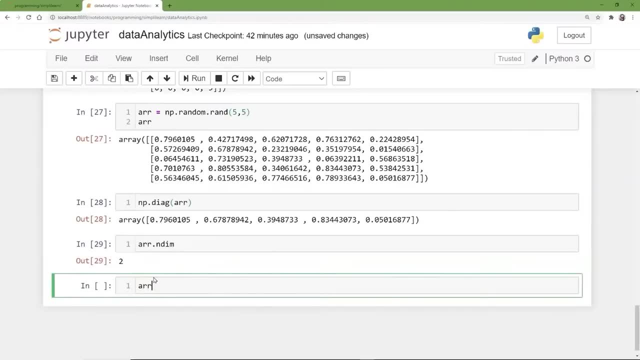 Print the shape out. You can also do the dimensions. So in dimensions very similar to shape It comes out and just has two dimensions. We can also look at the size. So if we do Size on here We can run that. 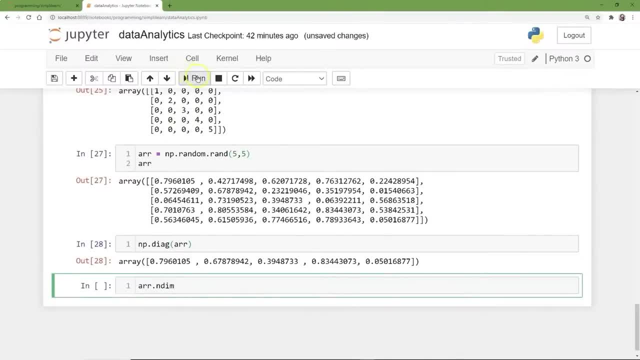 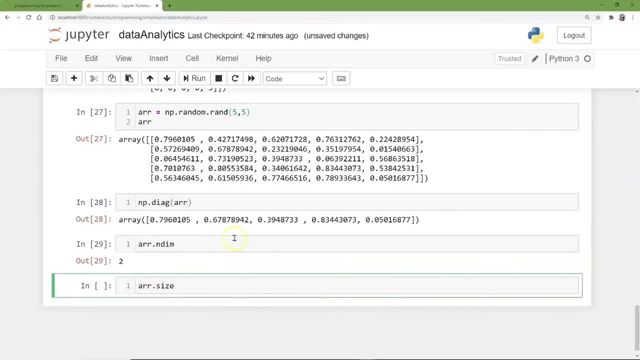 You can also do the dimensions. So in dimensions very similar to shape, it comes out and just has two dimensions. We can also look at the size. So if we do size on here, we can run that And you can see it has a size of 25,. 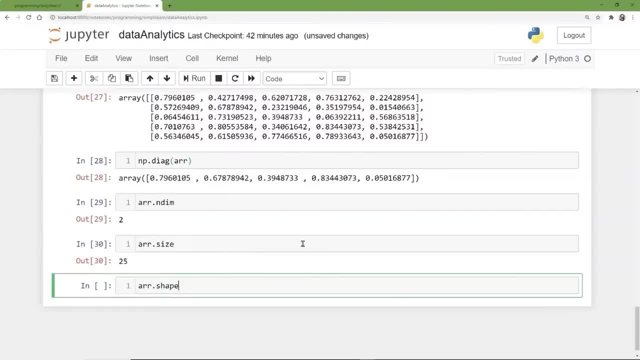 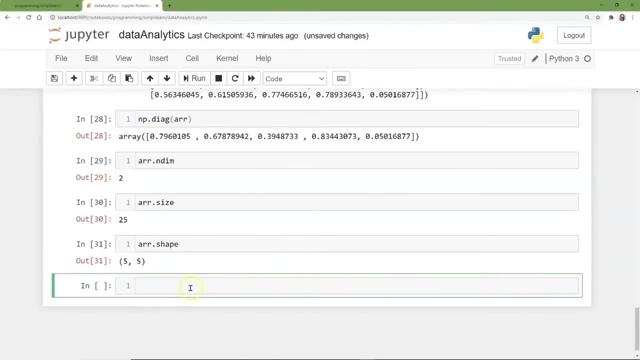 two dimensions and, of course, 5 by 5.. And that was from the shape from earlier that we looked at. There's our 5 by 5 shape And, if you remember, earlier we did random. Well, you can also do. 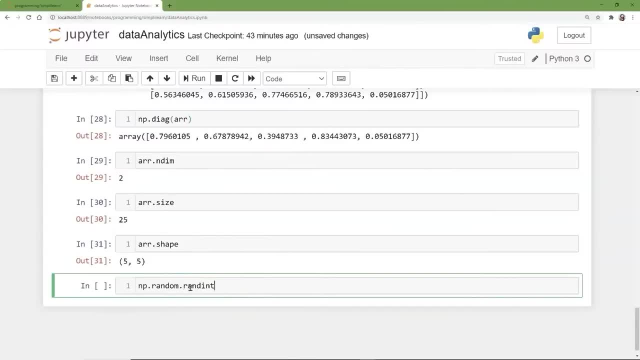 random. I talked a little bit about manipulating 0 to 1 and how you can get different answers. You can also do straight for the integer part And we'll do minus 10 to 10, 4. And so we're going to generate random integers. 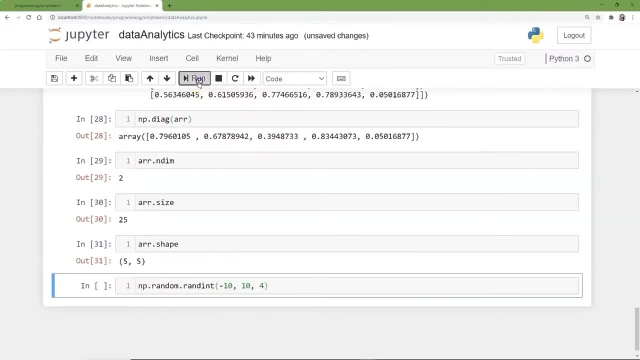 between minus 10 to 10.. We're going to generate four of those Once we run that. we have 7 minus 3 minus 6 minus 3.. They're all between minus 10 and 10.. And there's four of them. 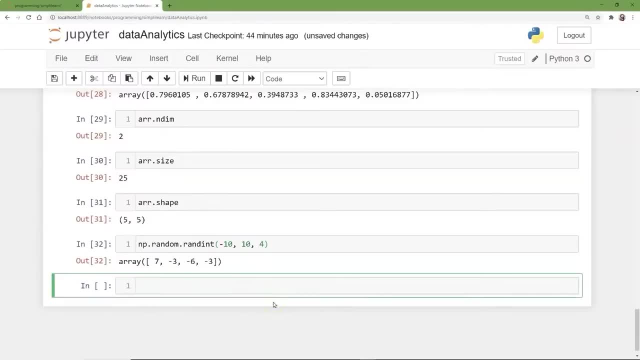 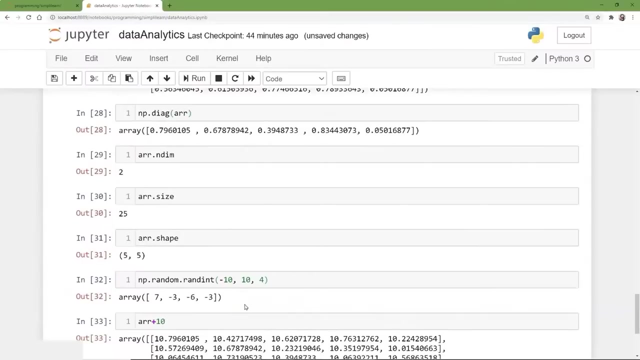 And now we jump into some of the functionality of arrays, which is really great because this is where they come in. Here's the array and you can add 10 to it, And if I run this there, it takes my original array from up here with the integers. 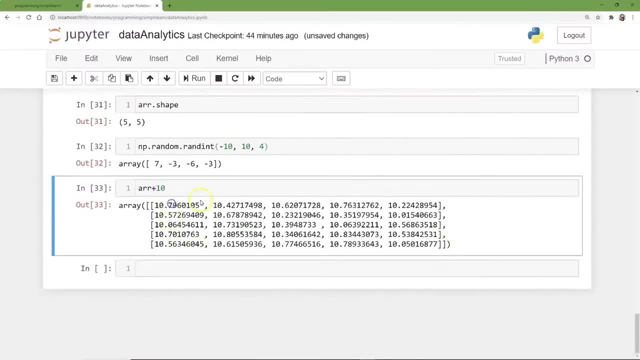 and adds 10 to all of those values. So now we have: oh, this is the decimal, That's right, This is a random decimal I had stored in array, But this takes the random numbers I had from 0 to 1. 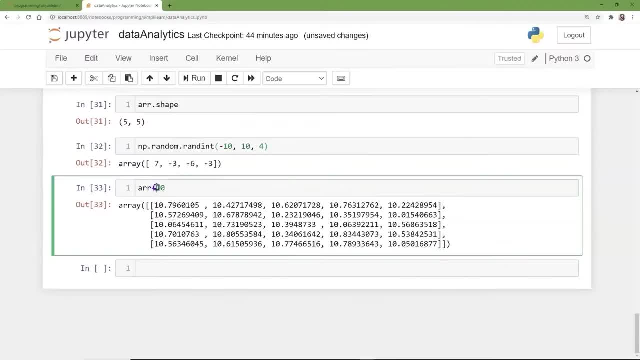 and adds 10 to them, And we can just as easily do minus 10.. We could even do times 2. And we could do divide by 2. And it'll take that random number we generated and cut it in half. So now all these numbers are under 0.5. 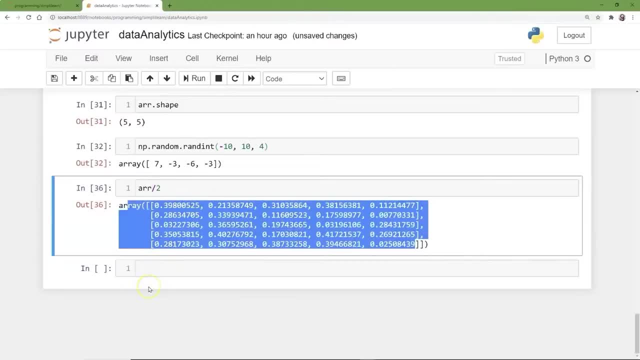 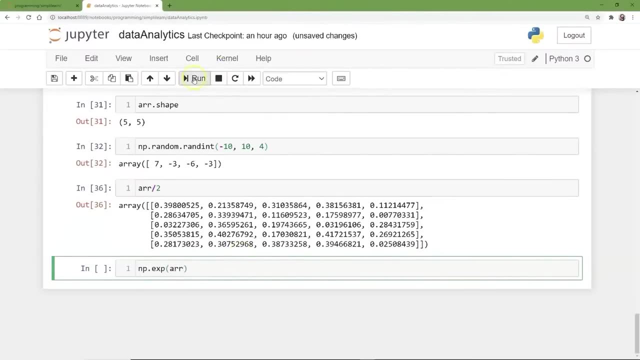 Another way you can change this. you can change the numbers to what you need on there And as you dig deeper into NumPy we can also do exponential. So as an exponential function which would generate some interesting numbers off of the random. 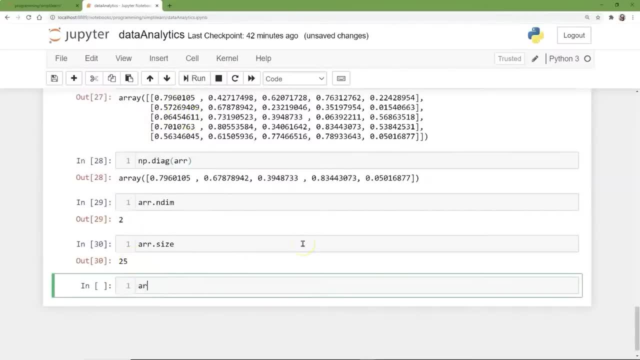 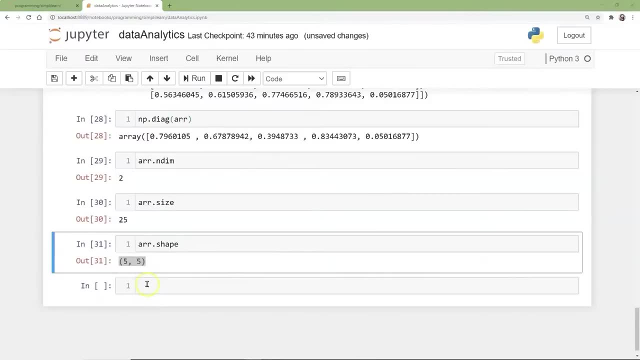 And you can see it has a size of 25.. Two dimensions And, of course, 5 by 5. And that was from the shape from earlier That we looked at. There's our 5 by 5 shape And, if you remember, earlier we did random. 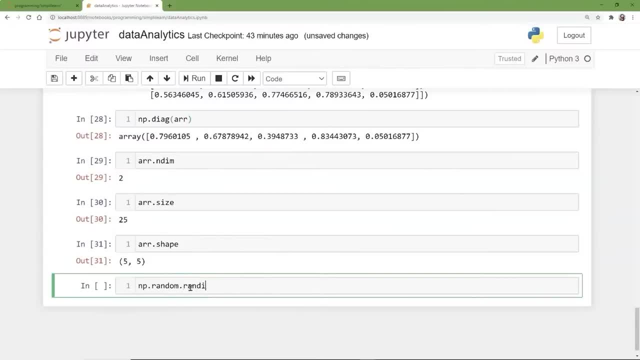 Well, you can also do random. I talked a little bit about manipulating 0 to 1. And how you can get different answers. You can also do straight for the integer part And we'll do minus 10. To 10. 4.. 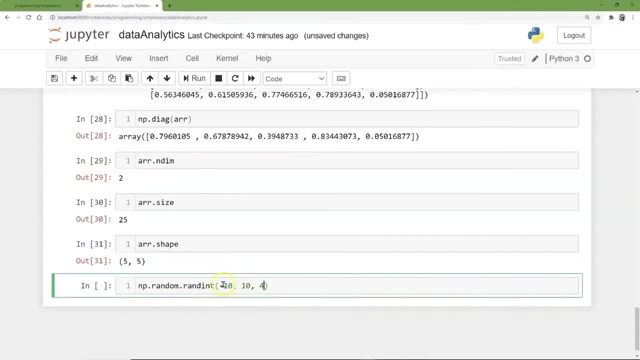 And so we're going to generate random integers Between minus 10 to 10.. We're going to generate four of those. Once we run that, we have 7 minus 3 minus 6 minus 3.. They're all between minus 10 and 10.. 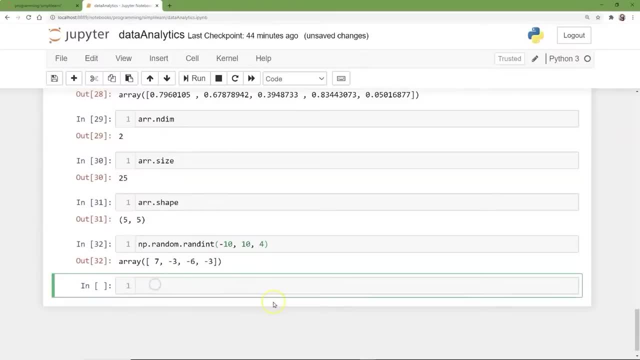 And there's four of them, And now we jump into some of the functionality of arrays, Which is really great Because this is where they come in. Here's your array And you can add 10 to it. And if I run this, 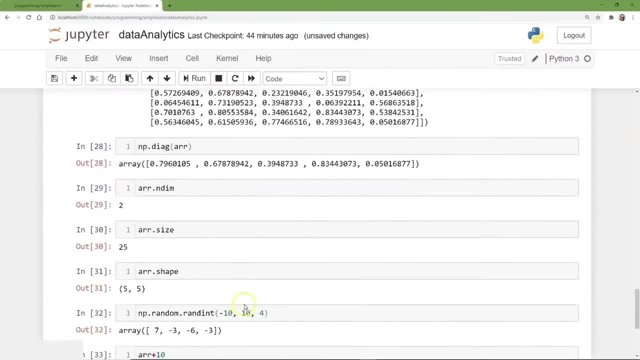 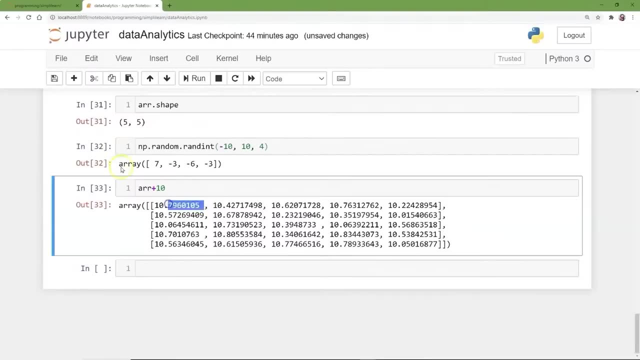 There. it takes my original array From up here With the integers And adds 10 to all of those values. So now we have: Oh, this is the decimal. That's right, This is a random decimal I had stored in array. 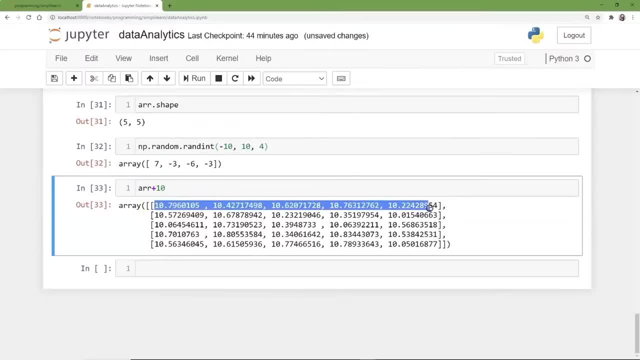 But this takes a random decimal, The random numbers I had, from 0 to 1. And adds 10 to them, And we can just as easily do Minus 10.. We could even do Times 2. And we could do divide by 2.. 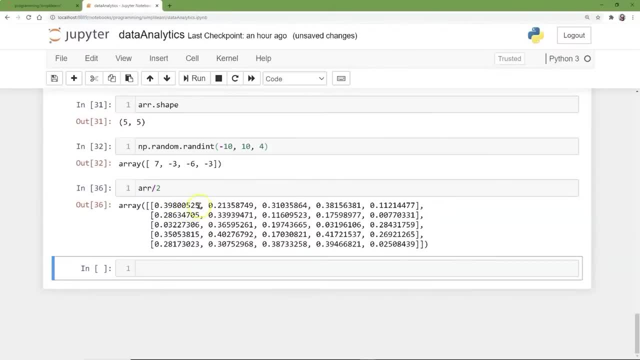 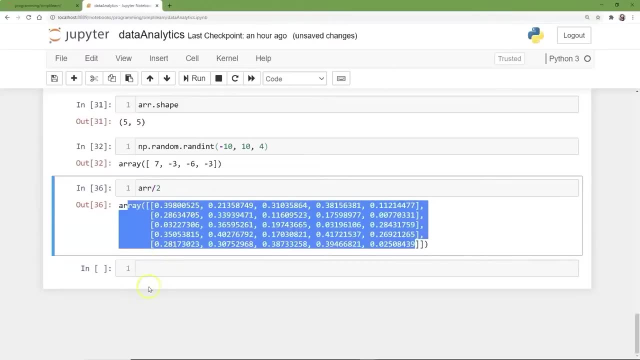 And it would. It'll take that random number we generated And cut it in half. So now all these numbers are under 0.5.. Another way you can Change the numbers to what you need on there And as you dig deeper into numpy. 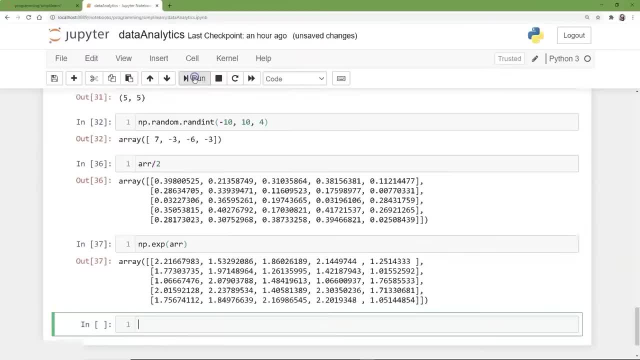 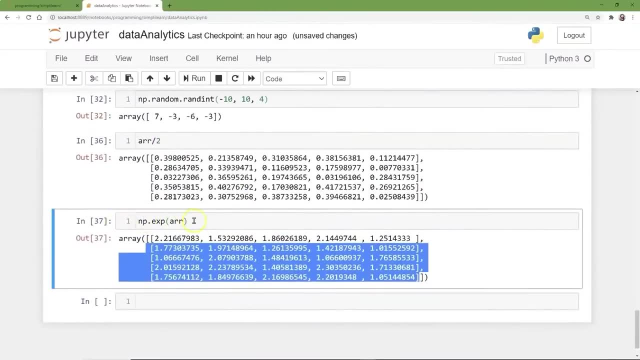 We can also do exponential, So as an exponential function Which would generate some interesting numbers off of the random. So we're taking them to the power. I don't even remember what the original numbers in the Array were, Because we did the random numbers up there. 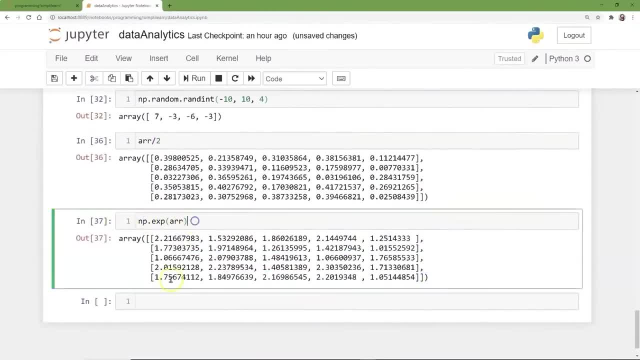 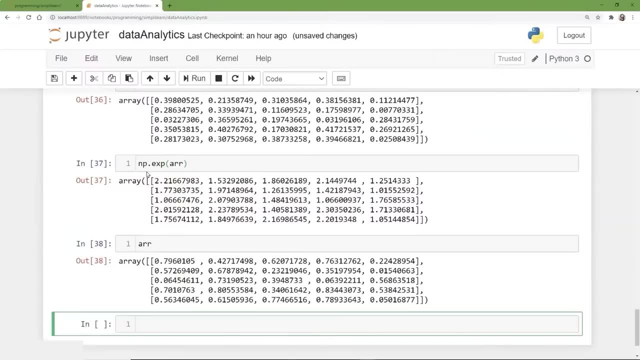 So we're taking them to the power. I don't even remember what the original numbers in the array were, because we did the random numbers up there. And here's our original numbers. And if you build an exponential on there, this is where you get e to the x on this. 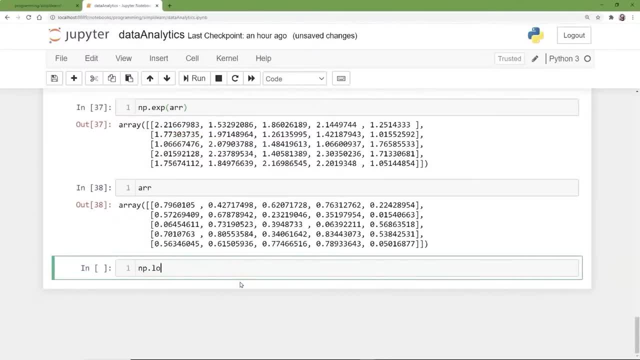 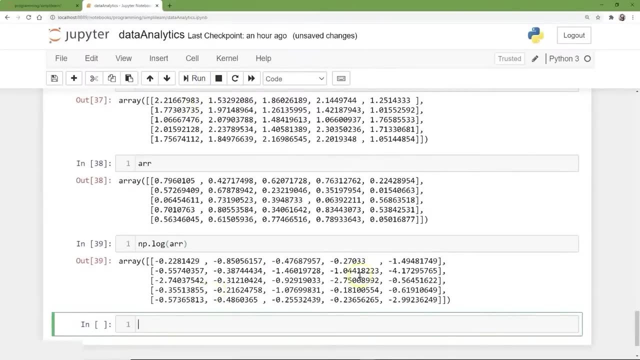 And just like you can do e to the x, you can also do the log. So if you're doing logarithmic functions that reinforce learning, you might be doing some kind of log setup on there And you can see the logarithmic of these different array numbers. 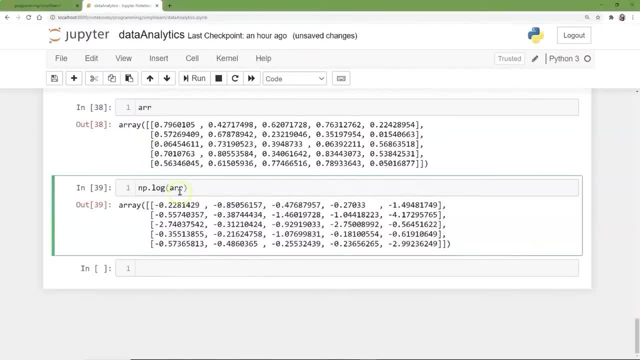 And if you're working with log base 2, you can just change it in there, np log 2.. You have to look it up because this is not log 1,, 2,, 3,, 4, 5.. It is log and log 2.. 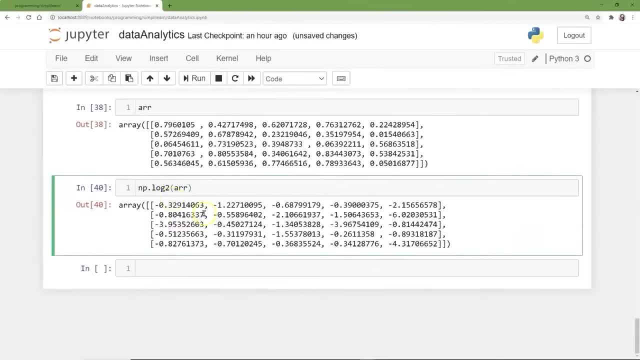 So just a quick note: this is not a variable going in, That is an actual command. There's a number of them in there and you'll have to go look and see what the documentation is, But you can also do log 10.. 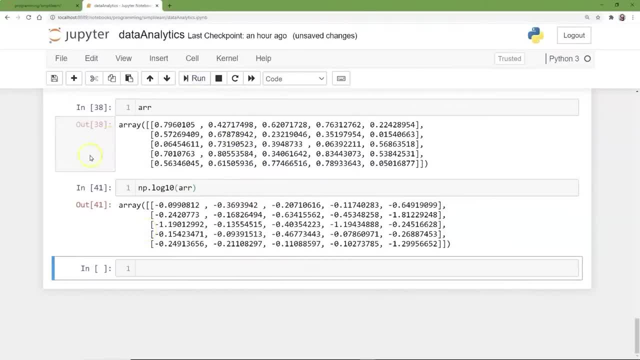 So here's log value 10. Some other really cool functions you can do with. this is your sine, So we can take a sine value of all of our different values in there. And if you have sine, you of course have cosine. We can run that. 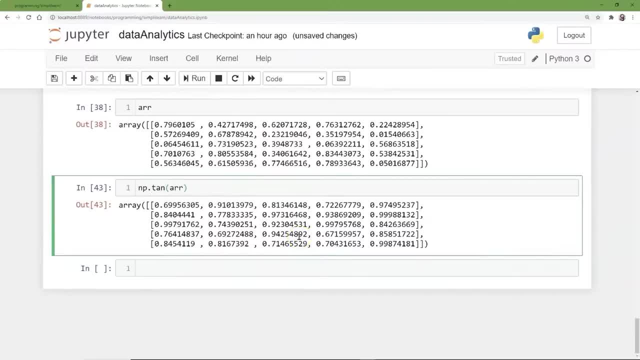 So here's the cosine of those, And if you're doing activations in your numpy array and you're doing a tangent activation, there's your tangent for that And the tangent activation is actually from neural networks. That's one of the ways you can activate it. 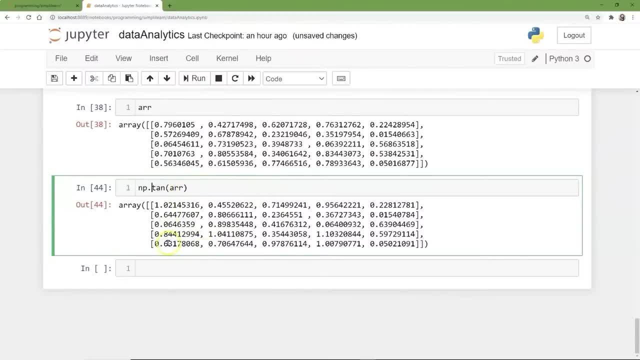 because it forms a nice curve from whether you're generating 1 to negative 1, with some discrepancy in the middle, Just jumping a little bit in there into neural networks, And then we get into. let me just put the array back out there so that we can see it. 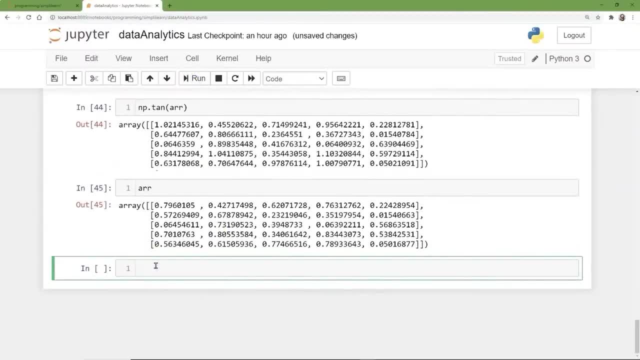 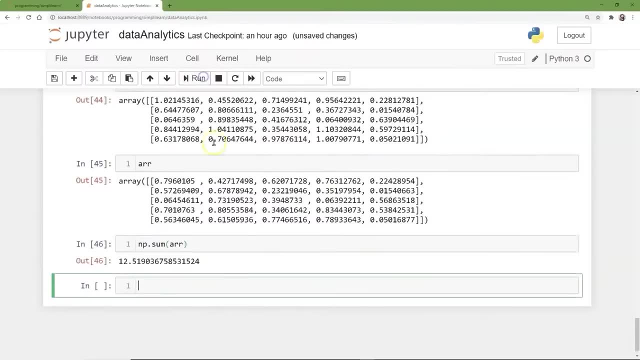 while we're doing this, As we're getting into this, you can also sum the values. So we have np sum And you can do a summation of all the values in this array And you'll see that if you added all these together, 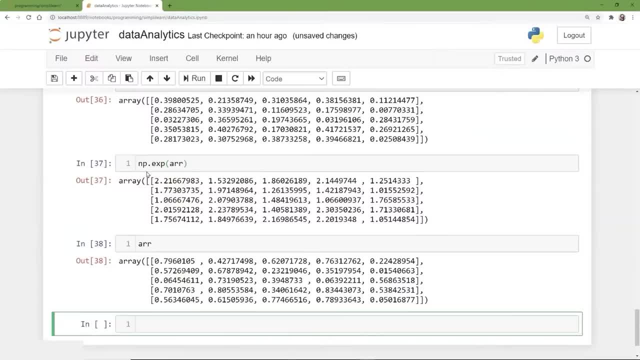 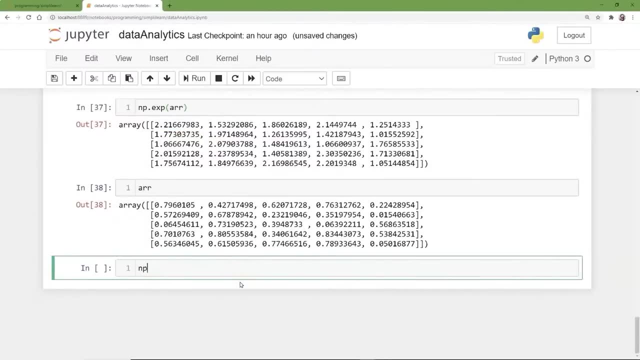 Here's our original numbers, And if you Build an exponential on there, This is where you get e to the x on this, And just like you can do e to the x, You can also do the log. So if we're doing logarithmic functions, 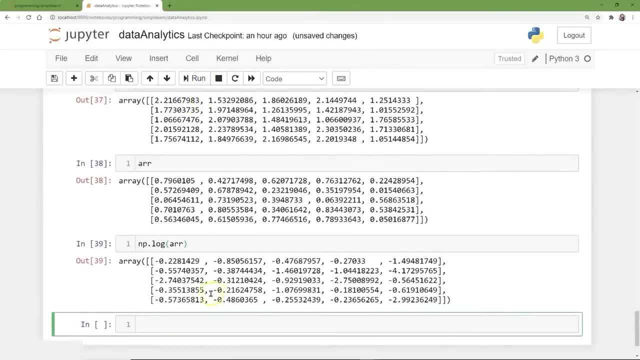 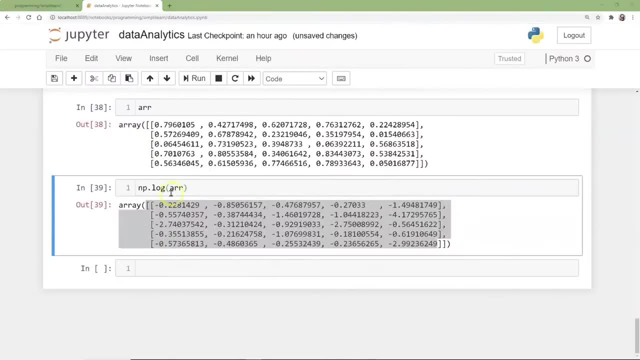 That reinforce learning. You might be doing some kind of log setup on there And you can see the logarithmic of these different array numbers. And if you're working with Log base 2.. You can do, You can just change it in there. 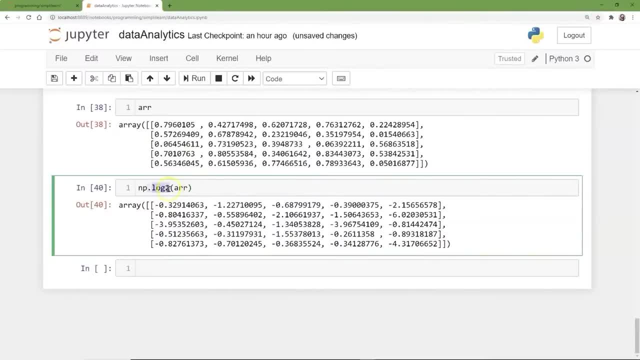 Np log 2.. You have to look it up Because this is not log 1, 2, 3, 4, 5. It is log and log 2.. So just a quick note, That's not a variable going in. 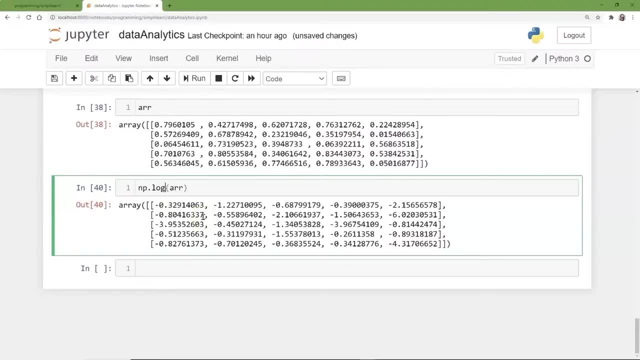 That is an actual command. There's a number of them in there And you'll have to go look and see What the documentation is. But you can also do log 10.. So here's log value 10. Some other really cool functions you can do with this. 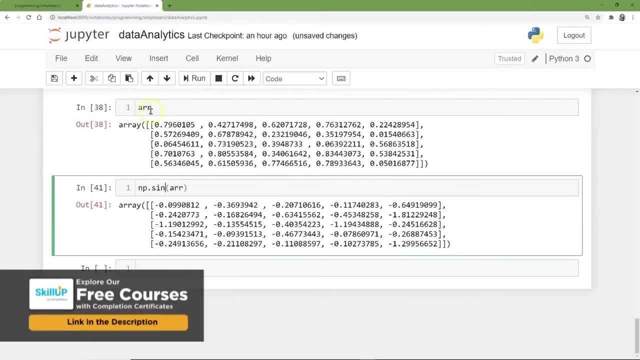 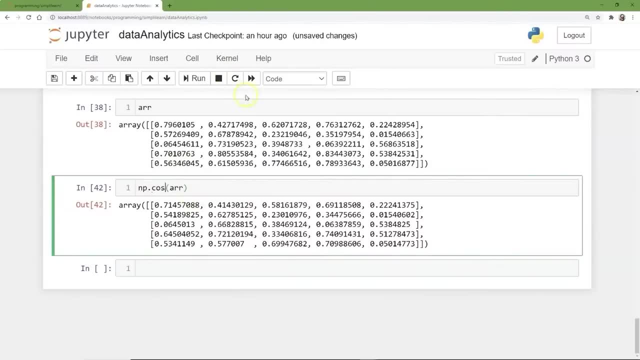 Is your sine. So we can take a sine value of all of our different values in there. And if you have sine, You of course have cosine. We can run that. So here's the cosine of those. And if you're doing activations, 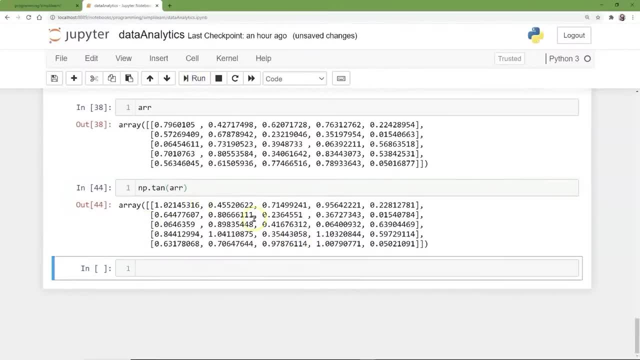 In your numpy array And you're doing a tangent activation. There's your tangent for that And the tangent activation is actually From neural networks. That's one of the ways you can activate it, Because it forms a nice curve between From whether you're generating 1 to negative 1.. 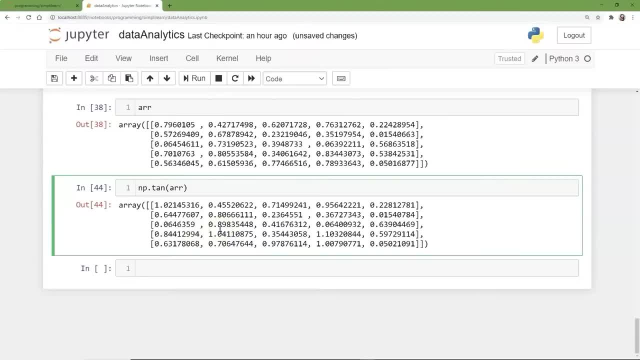 With some discrepancy in the middle, Just jumping a little bit in there Into neural networks, And then we get into. Let me just put the array back out there So that we can see it While we're doing this, As we're getting into this. 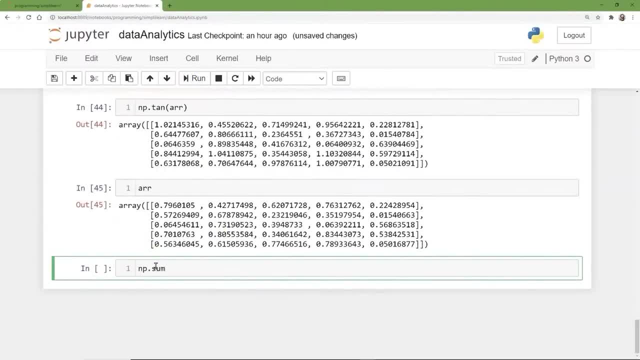 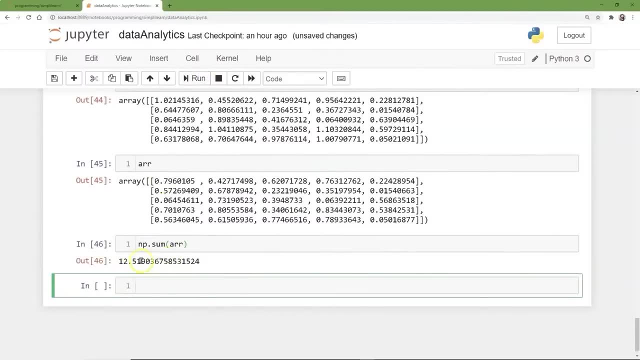 You can also sum the values. So we have np sum And you can do a summation Of all the values in this array And you'll see that If you added all these together They'd equal 12.519.. And so on. 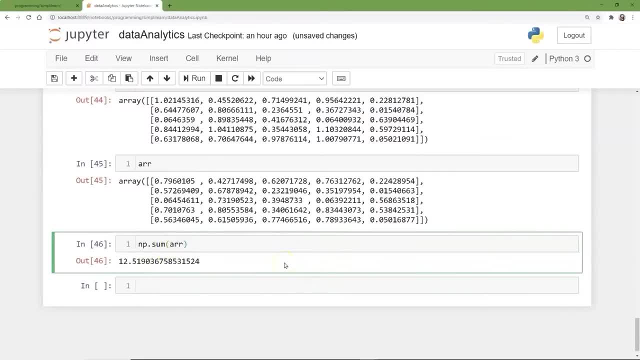 I don't know what the whole Setup is in there, But you can see right here The summation of this. One of the things you can also do Is by axes. So we can do: axes equals 0. And if we run, 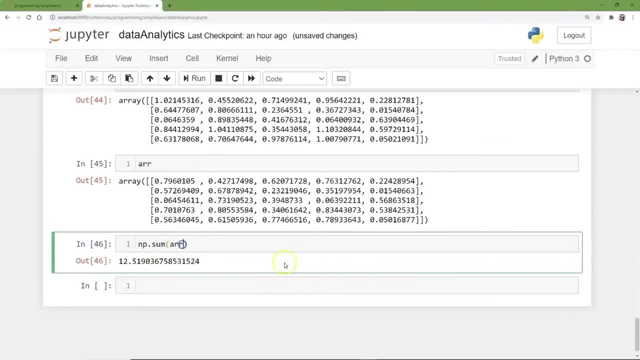 they'd equal 12.519 and so on. I don't know what the whole setup is in there, But you can see right here the summation of this. One of the things you can also do is by axes, So we can do axes equals 0.. 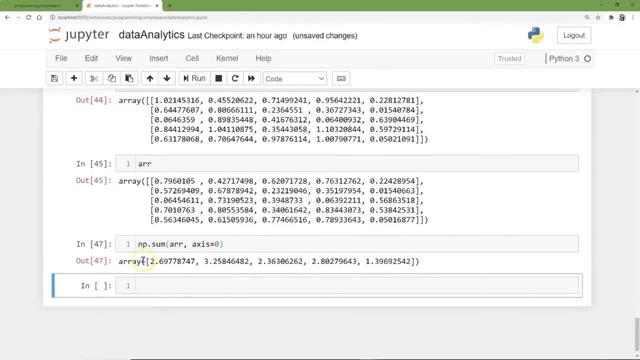 And if we run, the summation of the axes equals 0.. And you can think of that in numpy as the rows. So that would be. or you can think of that in numpy as being the columns. We're summing these columns going across. 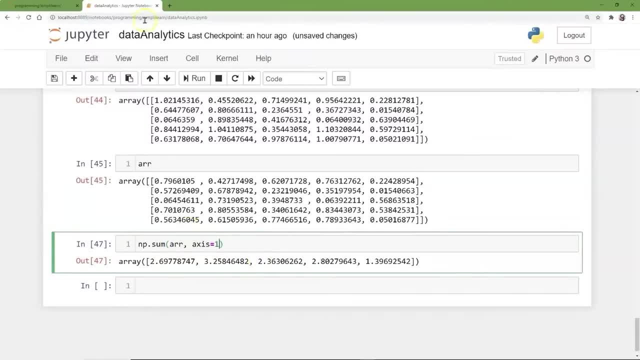 And you can also change this to 1.. And now we're summing the rows, And so that is the summation of this row and so forth and so forth going down, And maybe you don't need to know the summation, Maybe what you're looking for. 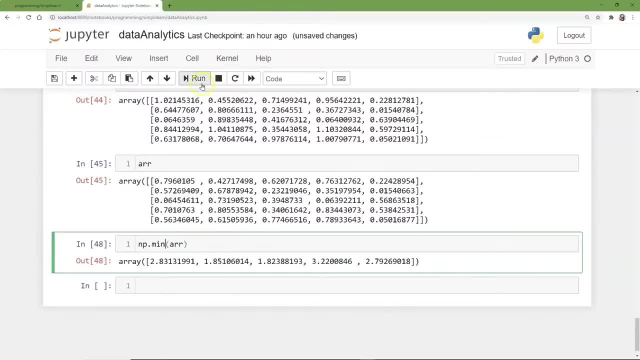 is the minimum. So here's our minimal You're looking for- and this comes up a lot because you have like your errors- We want to find the minimal error inside of this array And just like the other one we can do: axes equals 0.. 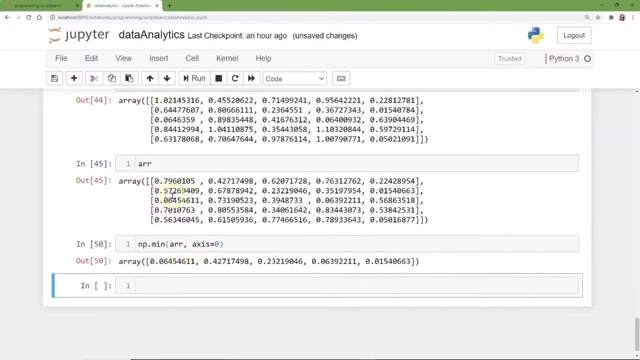 And you can see here, 0.0645 is the smallest number in this first column is 0.0645, and so on. And if you have a minimum, well you might also want to know the max. Maybe we're looking for the maximum profit. 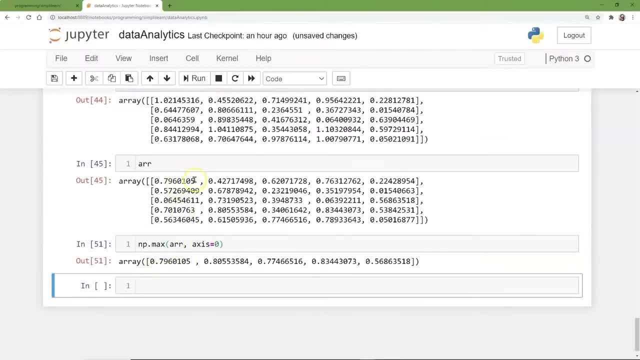 And here we go. You can see maximum. 0.79 is the maximum on this first column And, just like we did before, you can change this to a 1. on axes: You can take the axes out of here and just find the max value for the whole array. 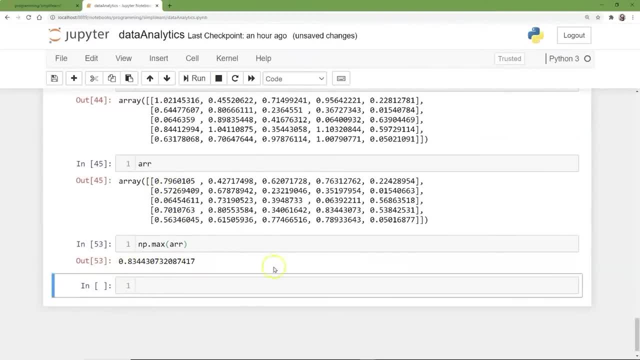 And the max value in here was 0.8344, so on and so on, And since we're talking data analytics, we want to go ahead and look at the mean. Pretty much the same as the average. This is the mean across the whole thing. 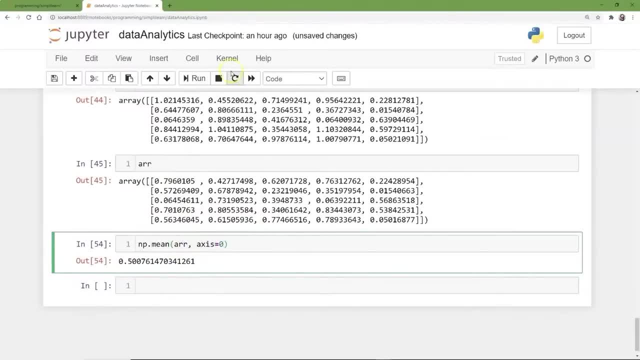 And just like we did before, we could also do axes equals 0. And then you'll see, this is the mean of this axis and so on, And we have mean We might want to know the median, And there's our median, our most common numbers. 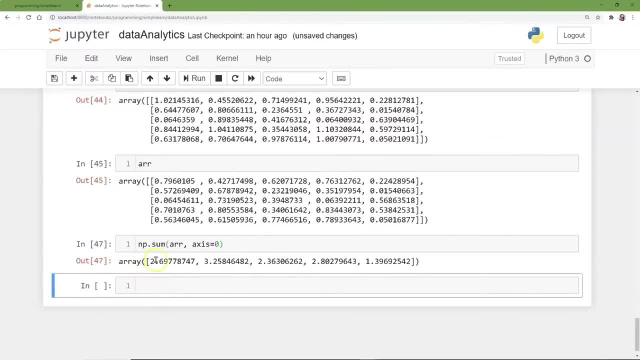 The summation of the axes equals 0.. And you can think of that In numpy As the rows. So that would be, Or You can think of that In numpy As being the columns. We're summing these columns. 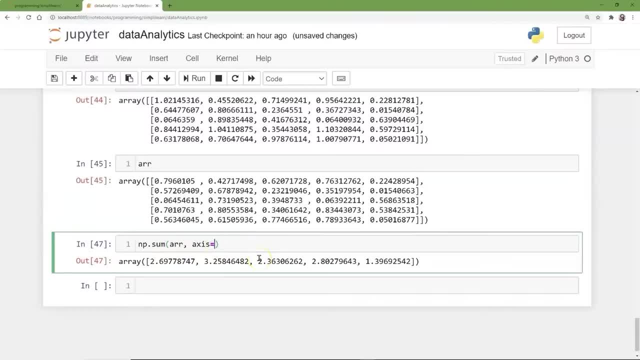 Going across, And you can also change this to one, And now we're summing the rows, And so that is the summation of this row, And so forth And so forth Going down, And maybe you don't need to. 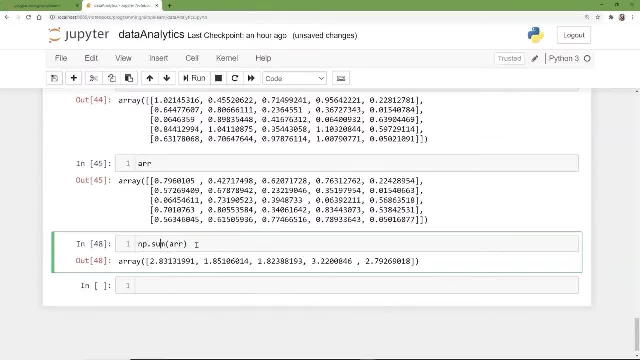 Know the summation. Maybe what you're looking for Is the minimum. So here's our minimal. You know You're looking for- And this comes up a lot Because you have Like your errors- We want to find the minimal error. 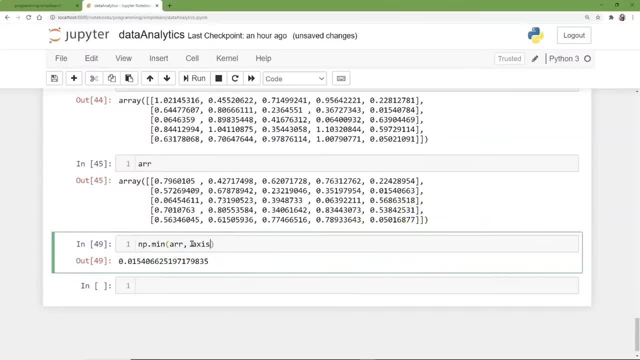 Inside of this array And just like The other one We can do, axes equals 0. And you can see here: 0.0645. Is the smallest number In this first column Is 0.0645.. And so on. 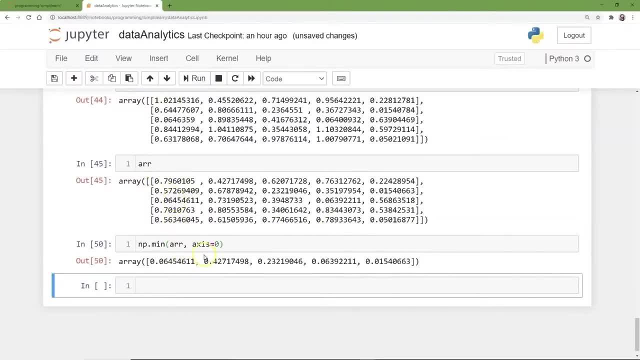 And if you have a minimum, Well, you might also Want to know the max. Maybe we're looking For the maximum profit And here we go. You can see The minimum Is 0.0645.. And so on. 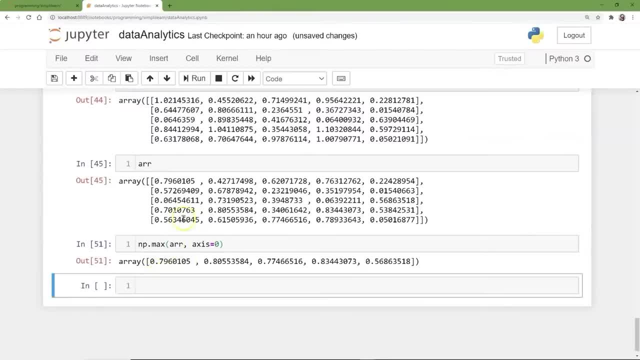 And if you have a minimum, And here we go, You can see Maximum: 0.79. Is the maximum On this first column And, just like We did before, You can change this To a 1.. On axes: 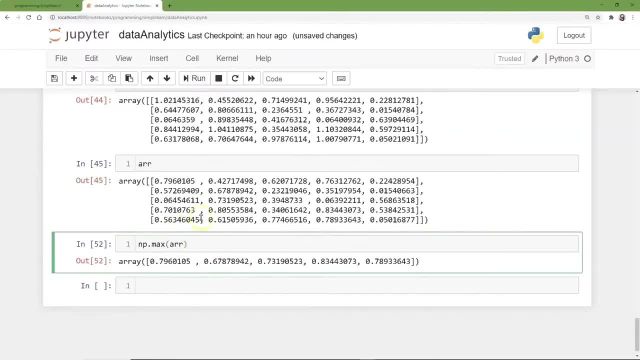 You can take the axes Out of here And just find the max Value For the whole array. And the max Value in here Was 0.8344.. So on, So on, And since We're talking, 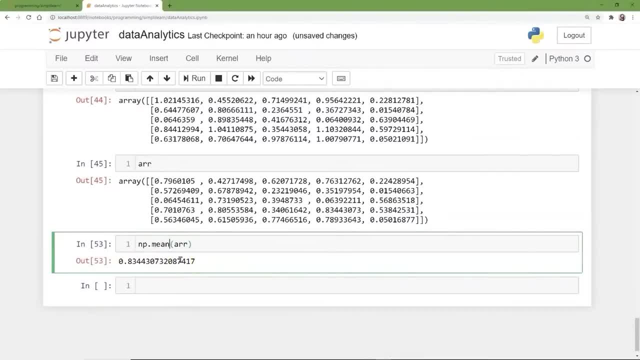 Data analytics. We want to go ahead And look at the mean. Pretty much the same As the average. This is the mean Across the whole thing. So, And just like We did before, We could also do: Axes equals 0.. 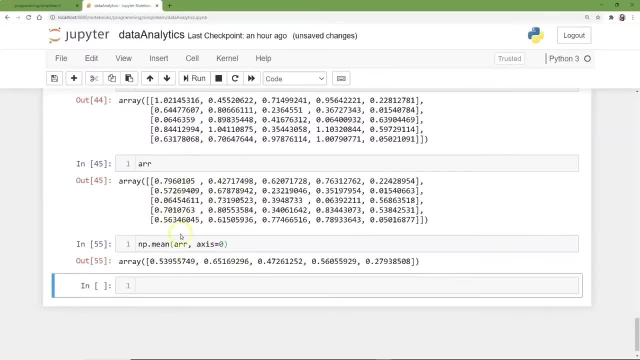 And then you'll see, This is the mean Of this axis And so on. And we have- mean We might want to know, The median. And there's our median, Our most common numbers. If we have median We might want to know. 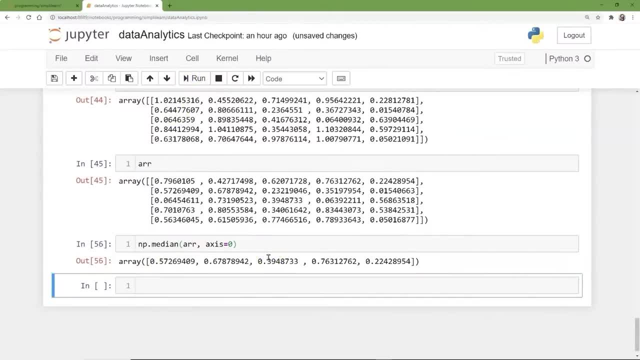 The standard deviation, Or If we have the average, A lot of times You do the means And the standard deviation. We can run that And there's our standard Deviations Along the axis Of the average And we can run. 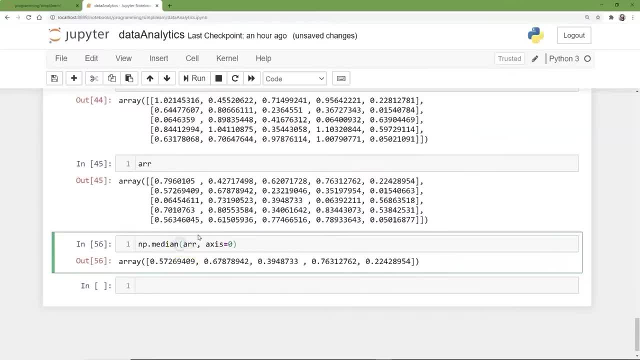 If we have median, we might want to know the standard deviation, Or if we have the average. a lot of times you do the means and the standard deviation. We can run that and there's our standard deviation along the axes. We can also do it across the whole array. 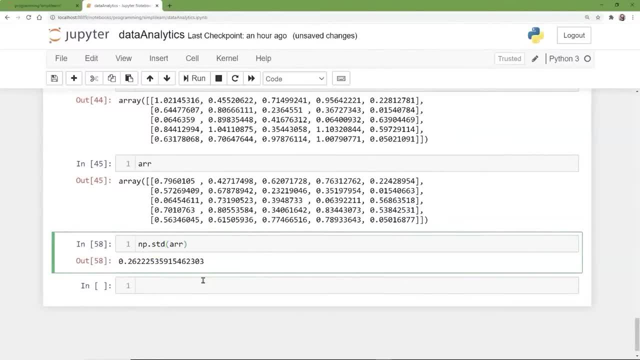 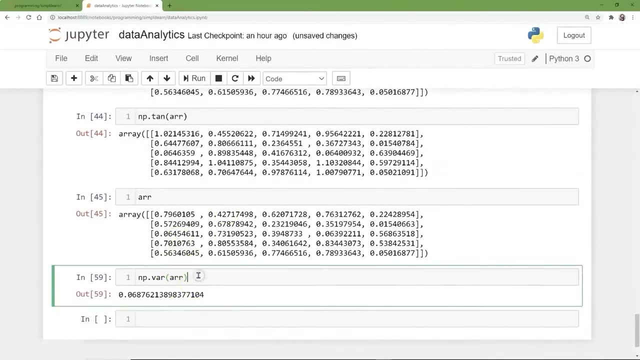 If we're going to do standard deviations, there's also variance, which is your VAR, And there's our variance across the data, Different levels, And so if we looked at that, we looked at variance, we looked at standard deviation, the median and the means. 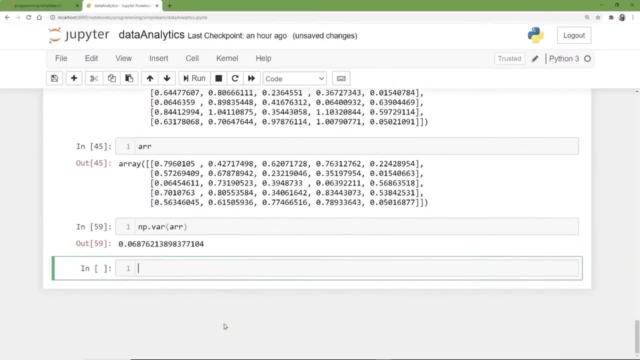 There's more, but those are the most common ones used. with data analytics And then going through your data and figuring out what you're going to present to the shareholders And some other things we can do, is we can actually take slices. You'll hear that terminology. 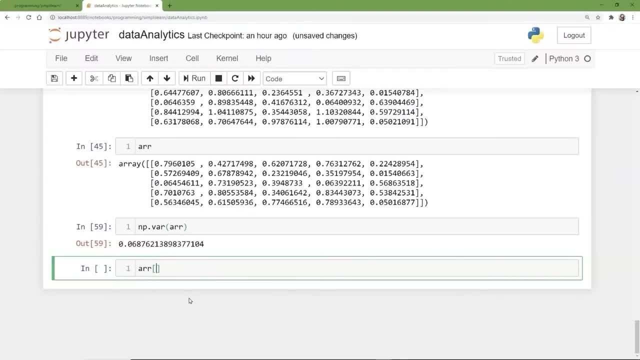 And a slice might be like: we have a five by five array, but maybe we don't want the whole array, Maybe we want from one on. we don't want the zero in there, So we got up to four And maybe on the second part. 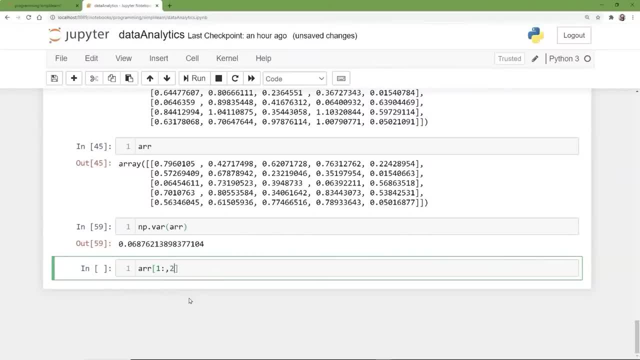 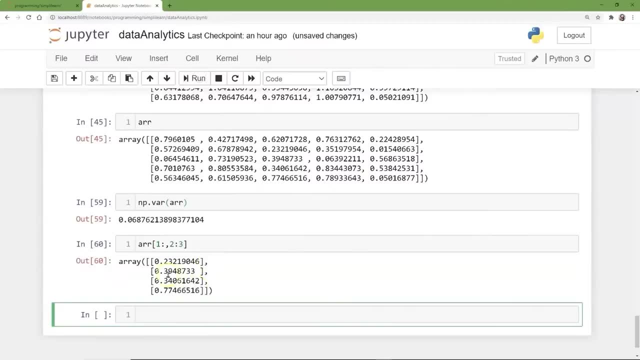 we just want two to row three, And so this notation right here says one to the end, And if we run this, you can see how that generates a single row to the end and then row two and three. Now, remember, it doesn't include three. 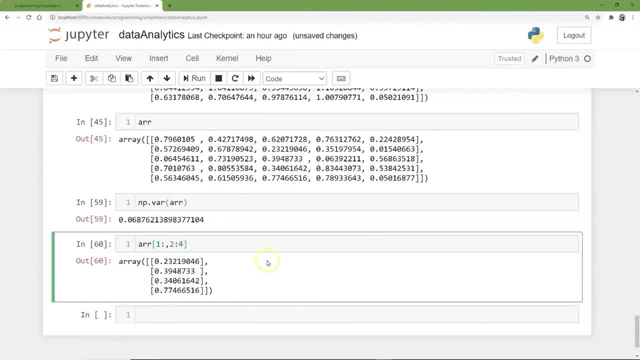 That's why we only get the one column. So if you wanted two and three, you would need to go ahead and go two to four, So it goes up to four. We could also do this in reverse, Just like we learned earlier. 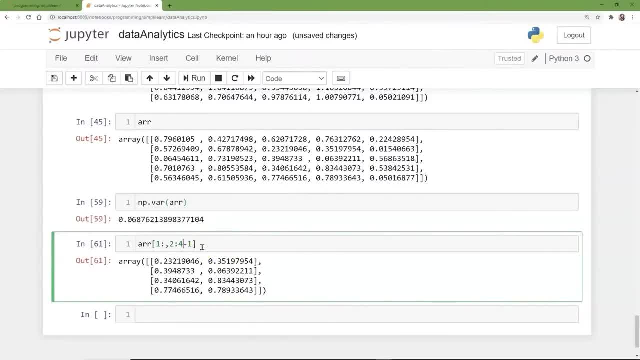 we can go minus one, Oops. And when we go to minus one, it's the same thing, because we have zero. one, two, three, four- This is the same thing as two to four. It goes two to the last one. 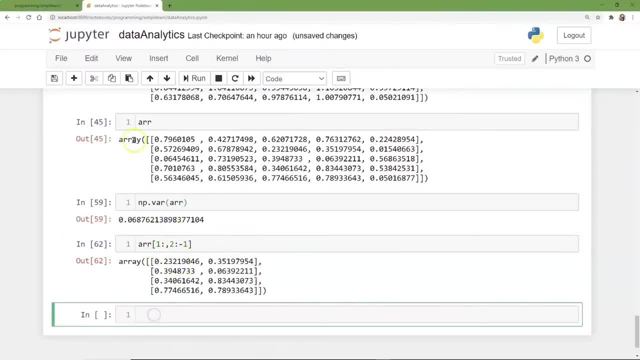 Also very common with arrays is you're going to want to sort them. So let's put our array up here that we randomly generated And we might want to sort it, And we'll go and throw an axis back in there. Axis equals one. 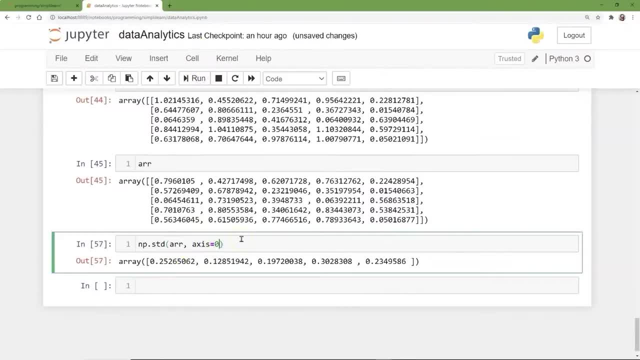 That And there's our standard Deviations Along the axis. We can also do it Across the whole array. If we're going to do Standard deviations, There's also Variants, Which is your VAR And there's our. 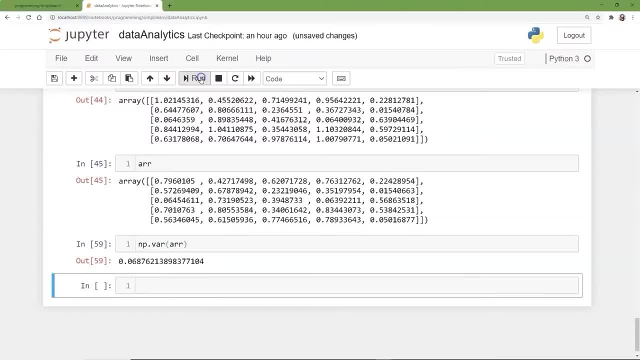 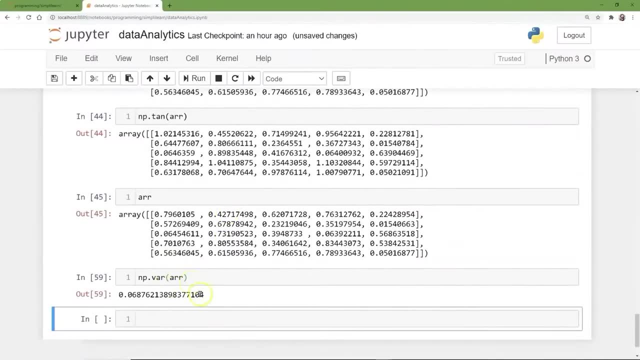 Variants Across the different Levels, And so If we looked At that, We looked At variance, We looked At standard deviation, The median And the means. There's more, But those are The most common. 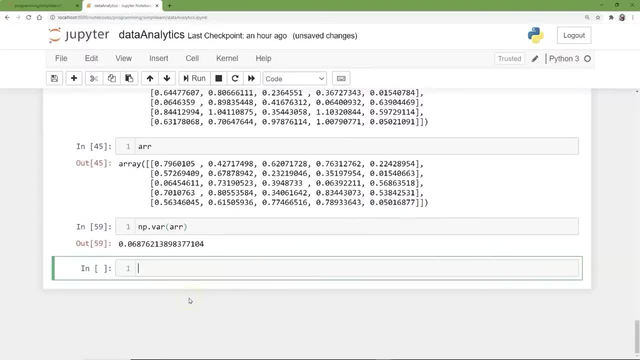 Ones Used With data analytics And then Going through your data Which are going to present To the shareholders. And some other things We can do Is we can actually Take slices- You'll hear That terminology And a slice. 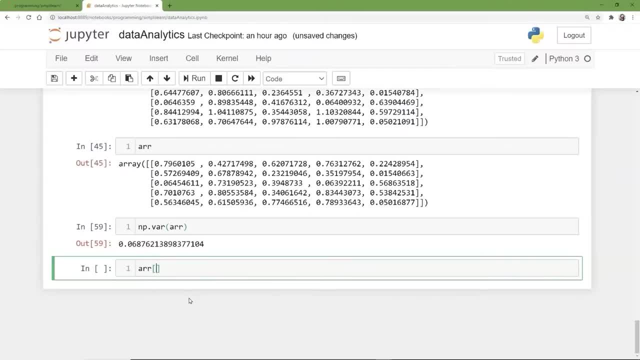 Might be Like we have A five by five array, But maybe We don't want The whole array, Maybe We want From one on. We don't want The zero in there, So we got Up to four. 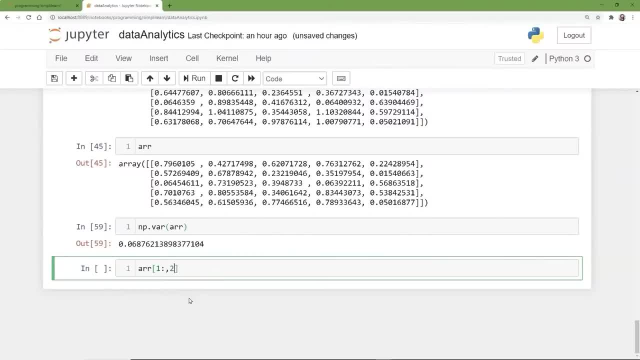 And maybe On the second part We just want Two To row Three And see This notation Right here Says One to the end And if we run this You can see How that generates A single row. 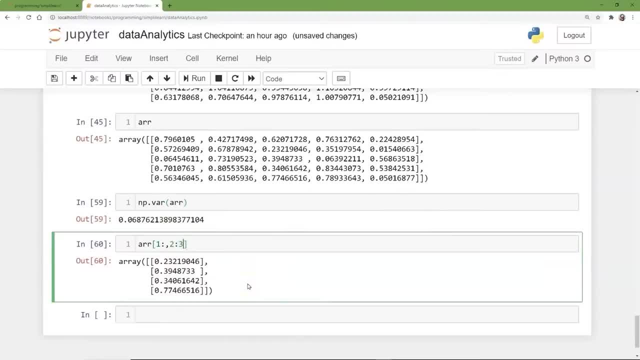 To the end And then row Two And three. Now remember It doesn't include Three. That's why We only get The one column. So if you wanted Two And three, You would need To go ahead. 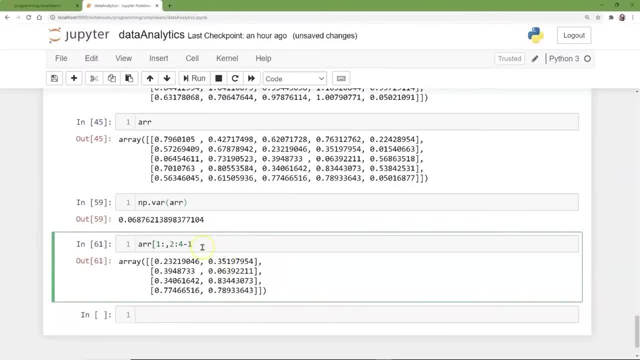 And go Two to four, So it goes Up to four. We could also Do this In reverse To minus One. It's the same thing, Because we have Zero, One, Two, Three, Four. This is the same thing. 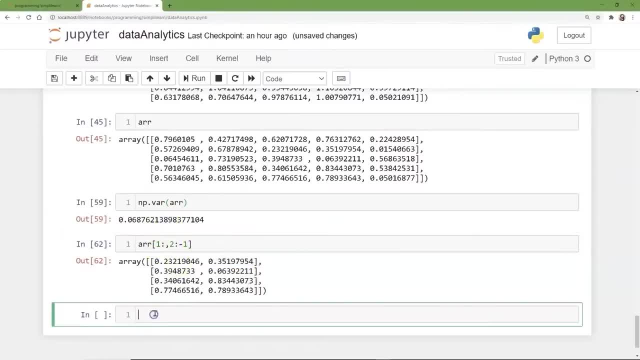 As two To four. It goes Two To the last One. Also very Common With arrays: Is you're going To want To sort Them? So we still have Our array Up here, That we. 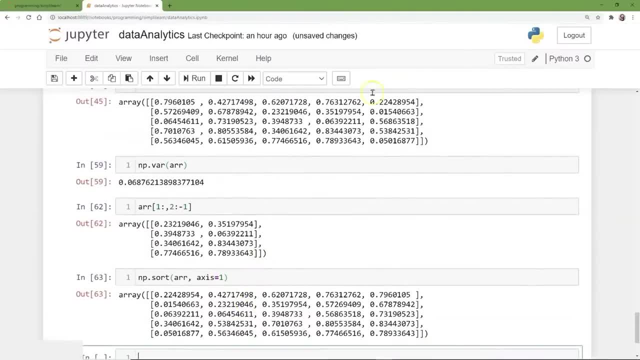 Randomly Generated This. You can see From the axes That it sorts It, The point Two Being the lowest Value To the highest Value By the row. We can also Change this, Of course. 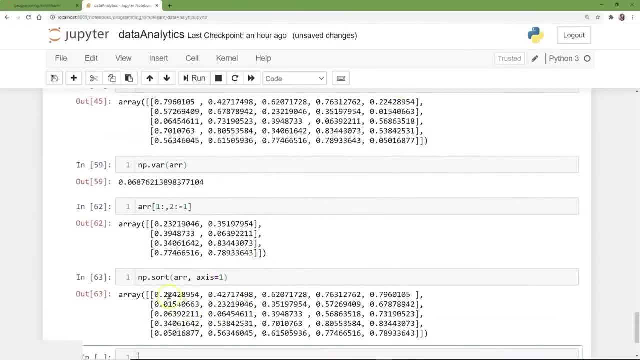 If we run this, you can see from the axes that it sorts it, the point two being the lowest value to the highest value by the row. We can also change this, of course, to axis zero If you're sorting it by columns. 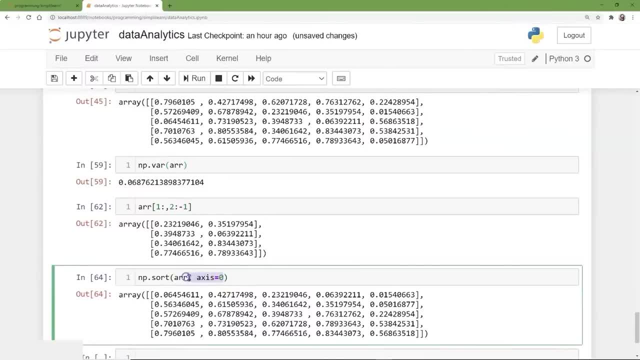 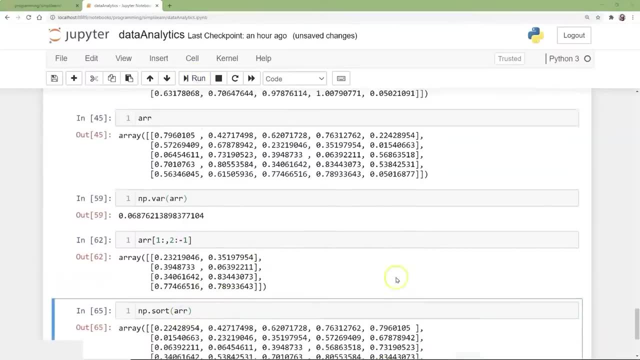 the values are based on columns, And then of course you can do the whole array And we can sort that. We don't usually do that, but you know, I guess sometimes that might come up And so you can see right here. 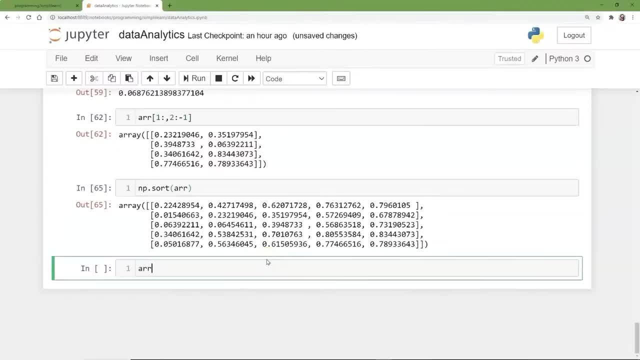 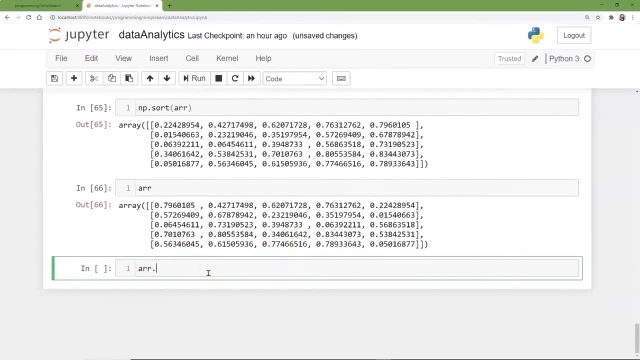 we have a nice sorted array. Something else? Let's just go ahead and reprint our array so we can look at it again, Starting to get too many boxes up there. Something else you can do with an array is we can take and transpose it. 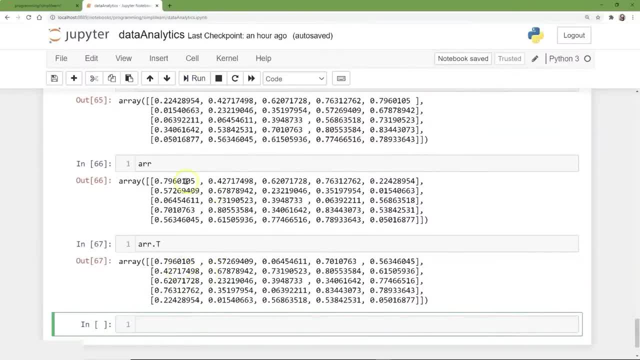 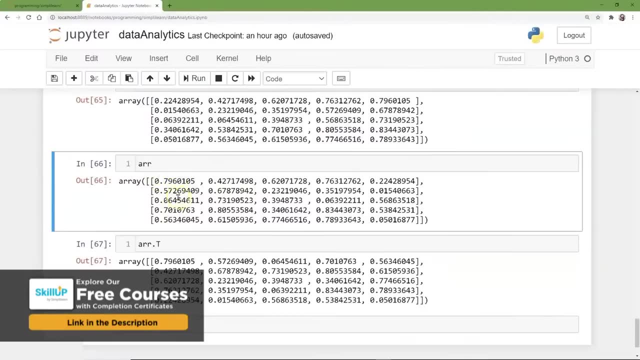 This comes up more than you would think. When you transpose it, you'll see that the rows and the column are transposed. So where 0.79, 0.57, 0.064 is the column, now we've switched it. 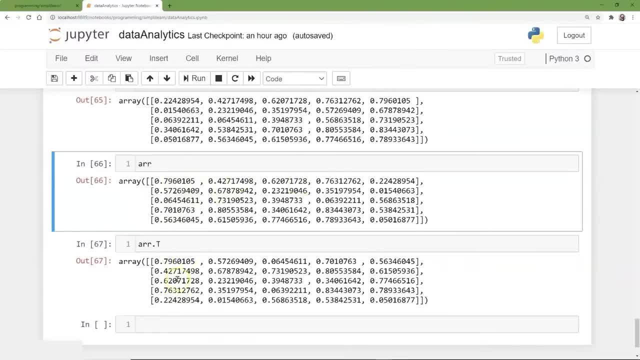 and we have 0.79, 0.42 as the index. You can see this really more dramatic if we take a slice, And we'll just do a slice- of the first couple And then we'll just do all the other. 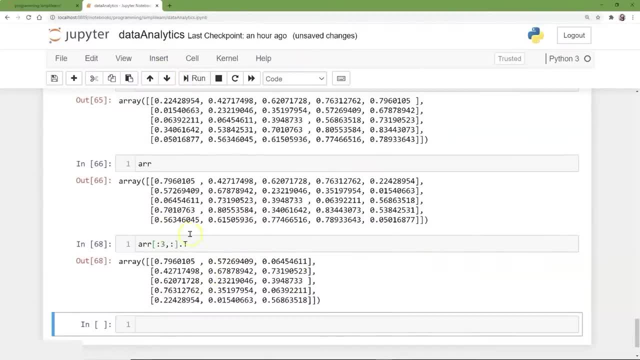 the full rows And if we run this, you can see how it comes up a little bit different, And we'll just do the same slice up here so you can see how those two look next to each other. There we go, There's our slice run. 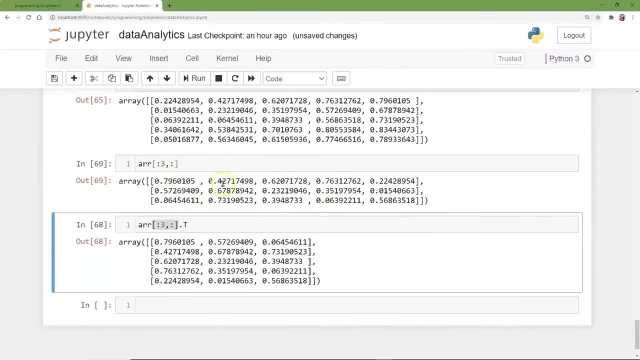 And so you can see the slice comes up and it has 1,, 2,, 3, 4, 5 columns. Now we have 1,, 2,, 3, 4, 5 rows and 3 columns versus 3 rows. 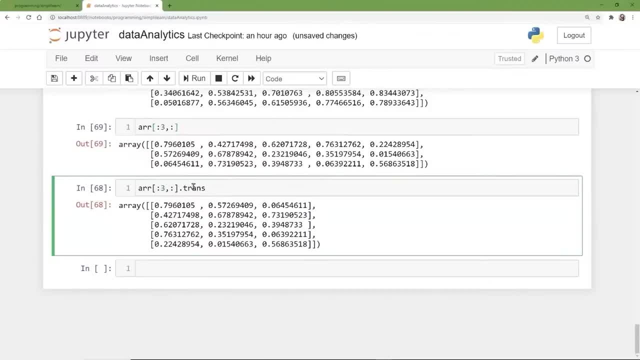 And the original version, when they first started putting this together, was a function. So the original version was transpose and this still works. You can still see it generates the same value as just a capital T. So many times we flip this data because we'll have an xy value. 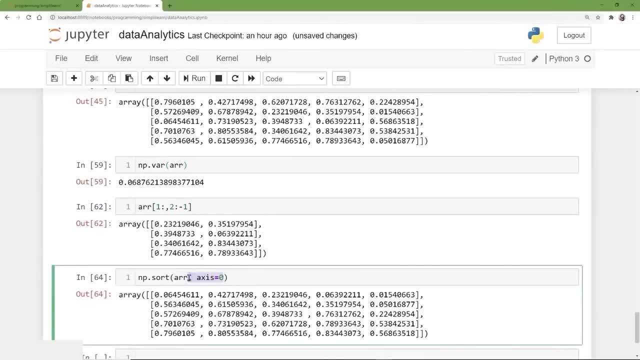 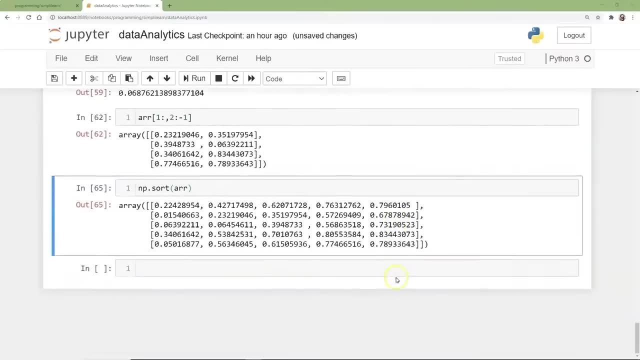 To axis Zero. If you're Sorting it By columns, So maybe Your values Are based On columns, And then, Of course, You can Do the whole Array Something. Now Let's just Go ahead. 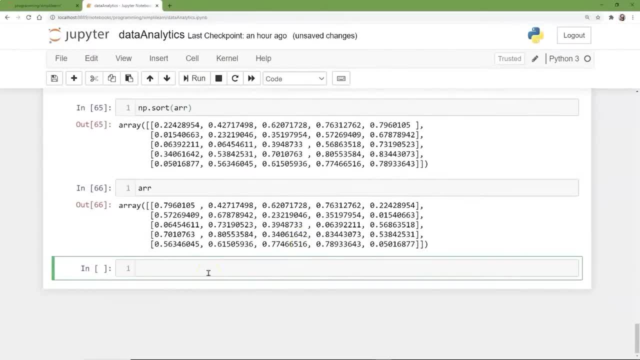 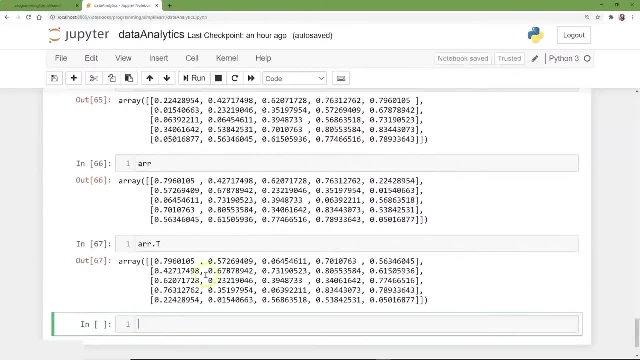 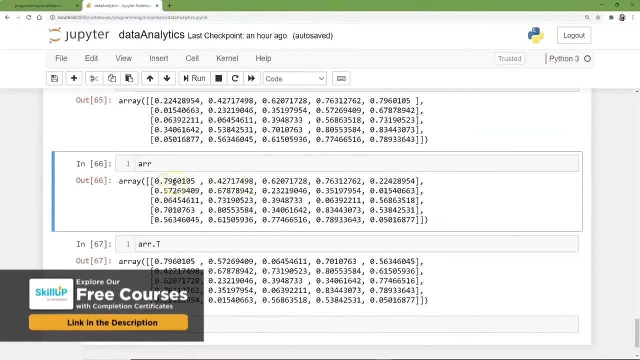 And reprint Our Array So we Can look At it Again, Starting To Get Too Many Boxes Up There. Something Else You Can Do With An Array Is 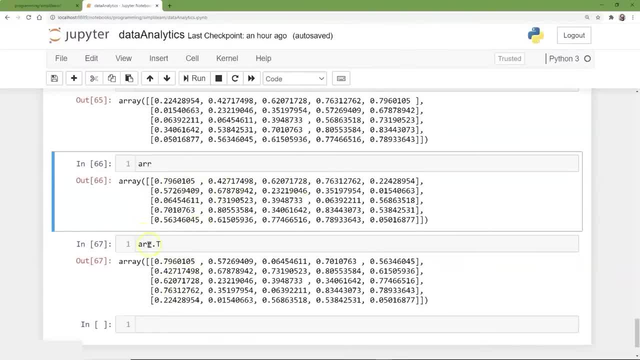 We Have Two As The Index. You Can See This Really More Dramatic If We Take A Slice- And We'll Just Do A Slice Of. 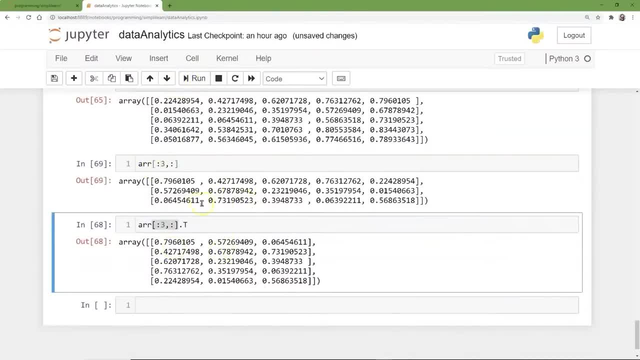 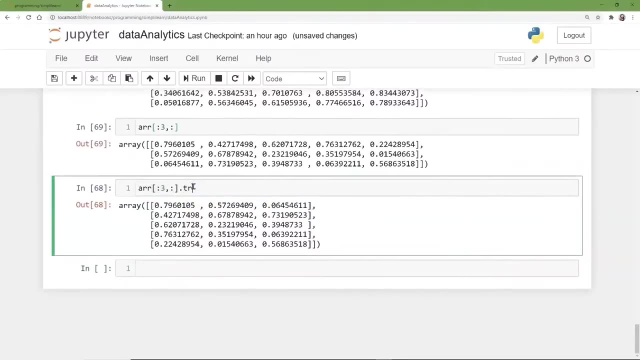 The First Couple, And Then We Have One, Two, Three, Four, Five Columns. Now We Have One, Two, Three, Four, Five Rows And Three Columns Versus. 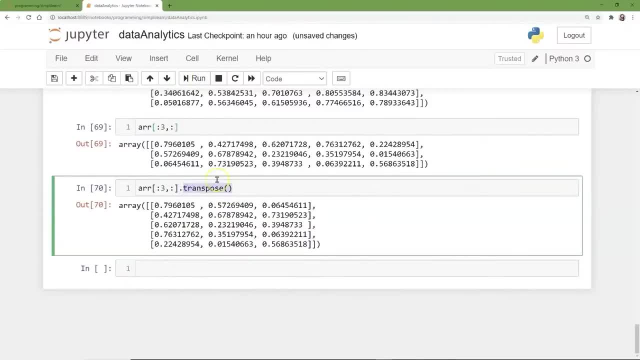 Three Rows And The Original Version, When They have an image or something like that and it's being read one way into the next process and the next one needs it the opposite. So this actually happens a lot. you need to know how to transpose the data really quick. 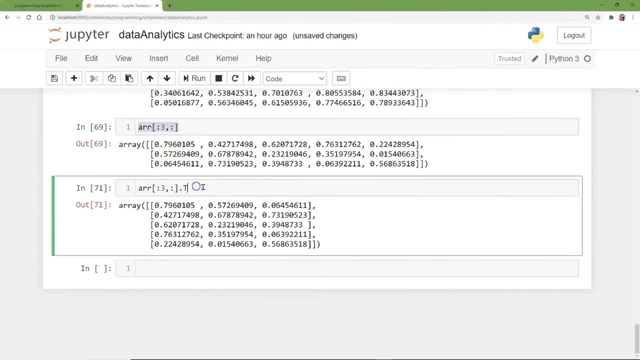 And we can go ahead. oh, let's just take here's our transpose. we'll just stick with the transpose on here and instead of doing it this way, we might need to do something called flattening. Why would you flatten your data? 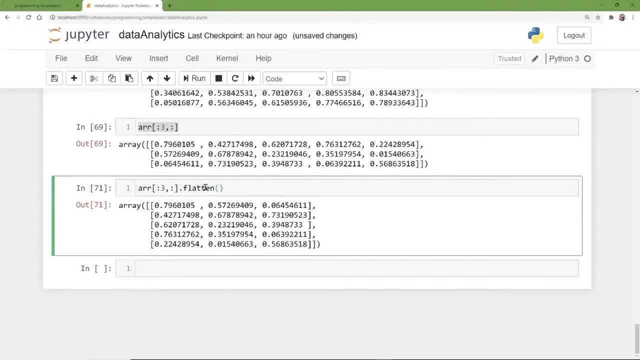 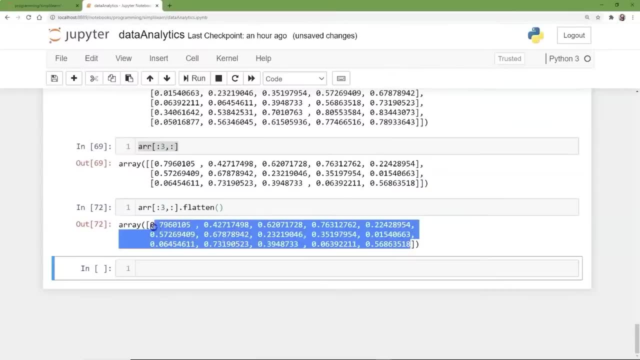 If this is an array going into a neural network, you might want to send it in as one set of values instead of two rows, And you can see here is all the values as a single array. it just flattens it down into one array. 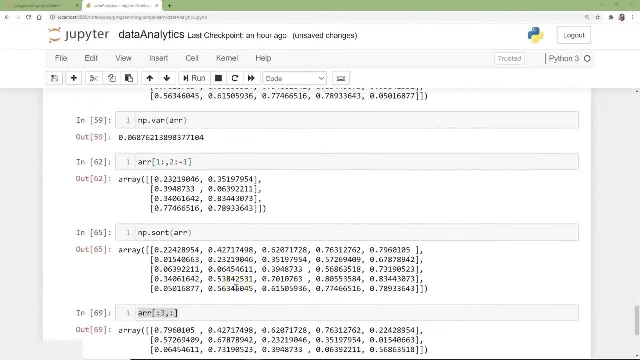 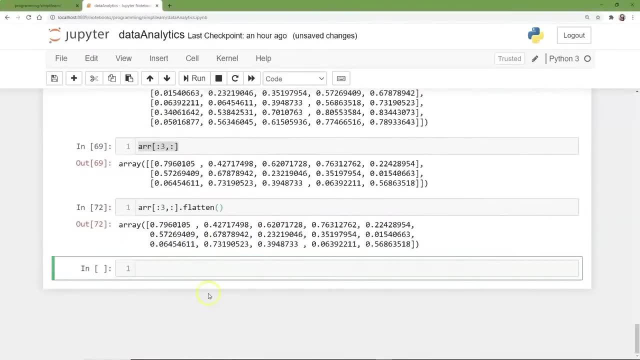 So we covered our scientific means: transpose, median, some different variations on here. Some of the other things we want to do is what happens if we want to append to our array. So let's create a new array. So let's create a new array. 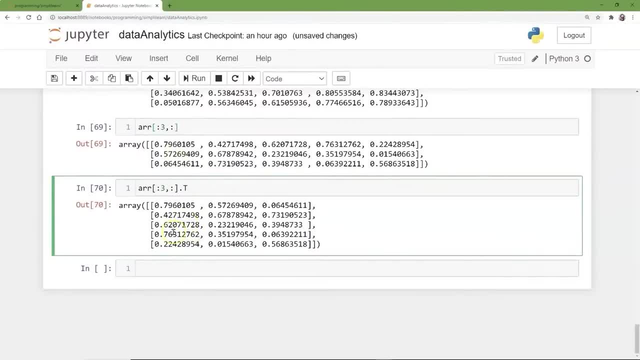 or we'll have an image or something like that and it's being read one way into the next process and the next one needs it the opposite. So this actually happens a lot. You need to know how to transpose the data really quick And we can go ahead. 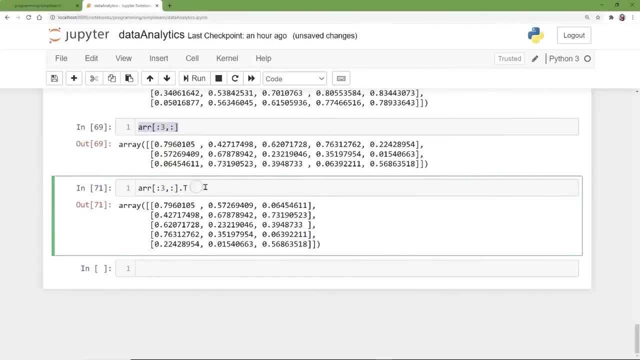 Oh, let's just take Here's our transpose. We'll just stick with the transpose on here, And instead of doing it this way, we might need to do something called flattening. Why would you flatten your data If this is an array going into a neural network? 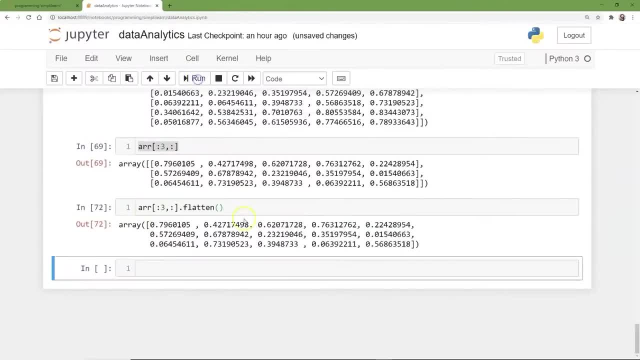 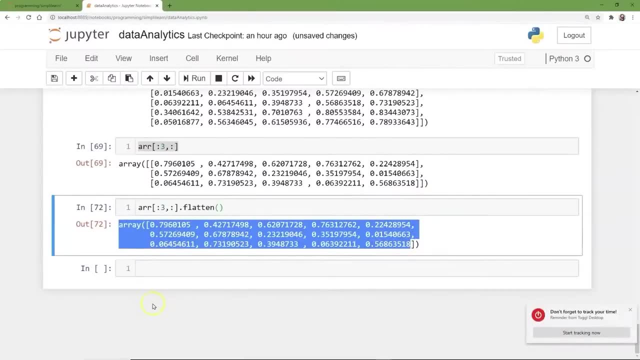 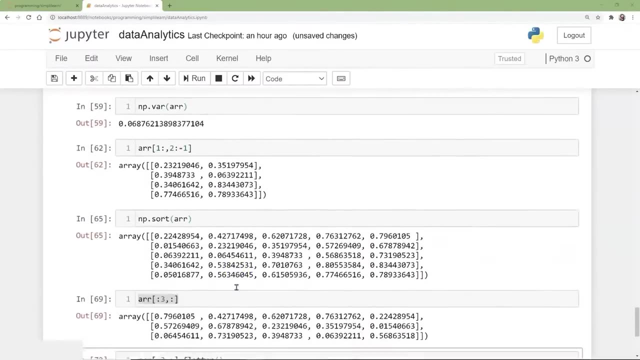 you might want to send it in as one set of values instead of two rows And you can see: here is all the values as a single array. It just flattens it down into one array. So we covered our scientific means: transpose median. 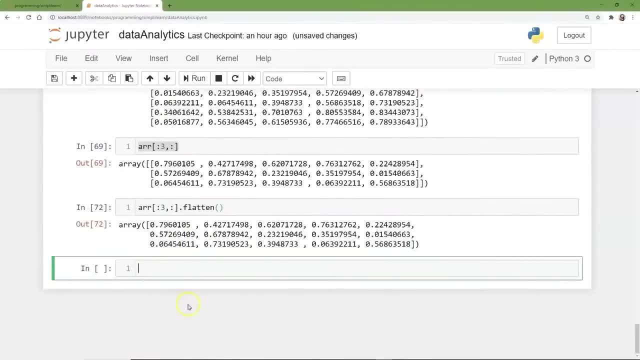 some different variations on here. Some of the other things we want to do is what happens if we want to append to our array. So let's create a new array. I'm getting tired of looking at the same set of random numbers we generated earlier. 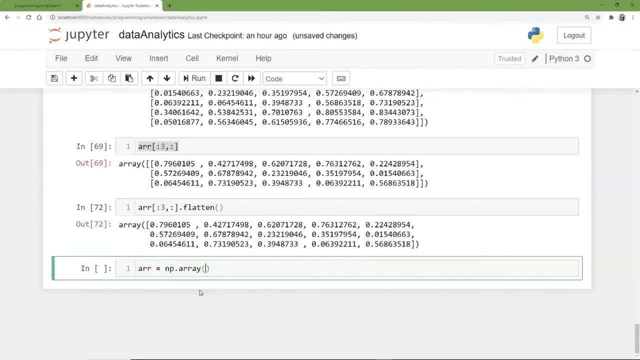 So we'll go ahead and create a new array here, something a little simpler so it's easier to see what we're doing. And four, five, six, seven, eight. That's good enough. We'll just do four, five, six, seven, eight. 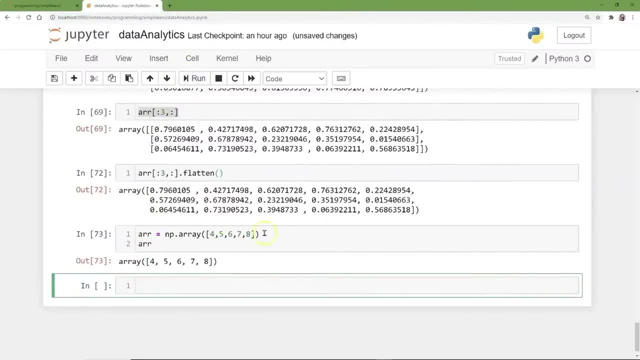 And if we print this array there it is four, five, six, seven, eight, And we might want to append something to the array. So we have our array. We need to extend it. You've got to be very careful. 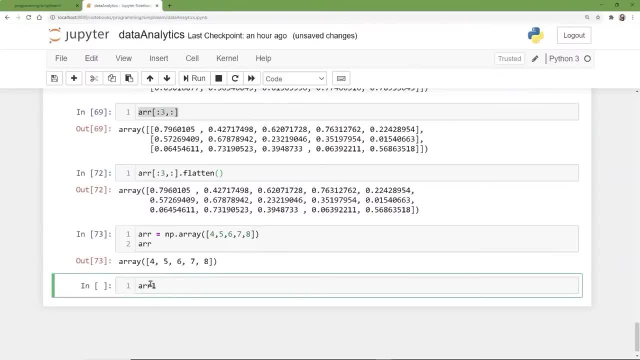 about appending things to your array, And there's a number of reasons for that. One is runtime, Because of the way the numpy array is set up. a lot of times you build your data and then push it into the numpy array instead of continually adding on to the array. 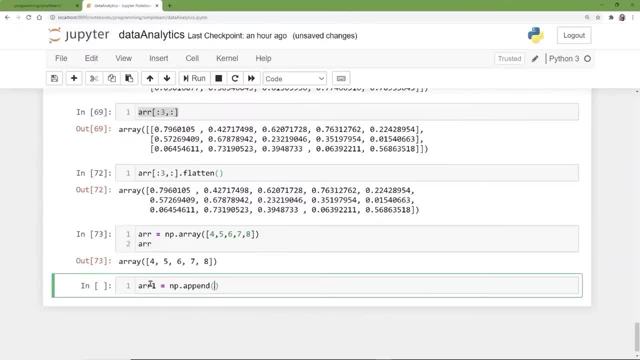 And then it also. usually it automatically generates a copy for protecting your data. So there's a lot of reasons to be careful about appending this way. But you can certainly do it And we can just take our array. We're going to create a new array, array one. 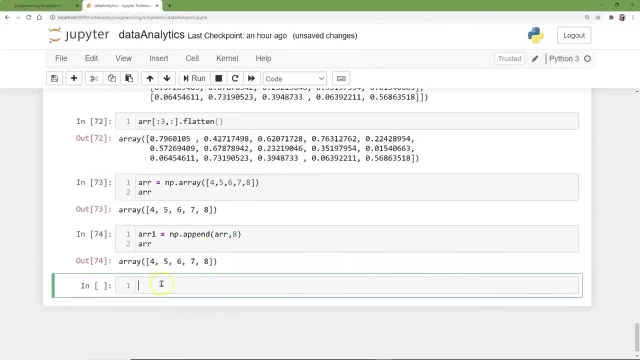 And if we print array one and we append eight to it, you'll see four, five, six, seven, and then there's our eight appended on to the end. And if you want to append something to an array, you'd probably also want to. 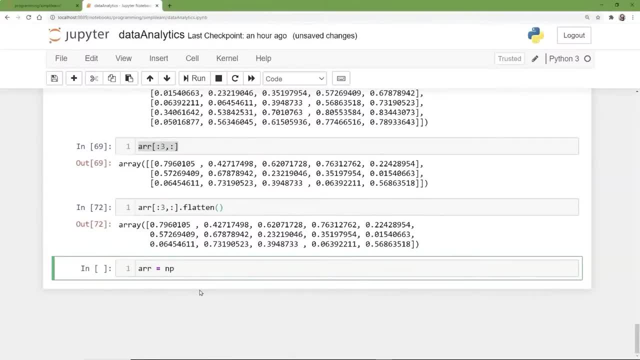 We're getting tired of looking at the same set of random numbers we generated earlier, So we'll go ahead and create a new array here, something a little simpler so it's easier to see what we're doing. And 4,, 5,, 6,, 7,, 8, that's good enough. we'll just do 4,, 5, 6,, 7, 8.. 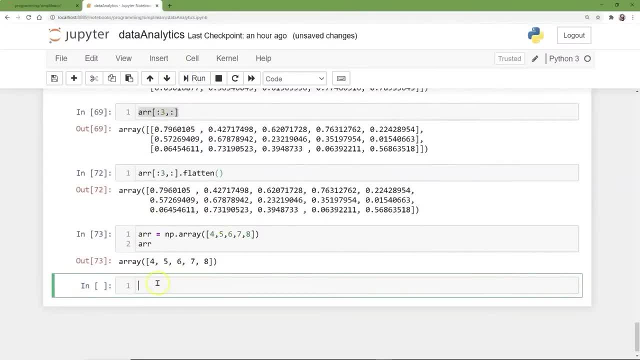 And if we print this array there, it is 4,, 5,, 6,, 7,, 8.. And we might want to append something to the array. So we have our array. we need to extend it. You've got to be very careful about appending things to your array and there's a number. 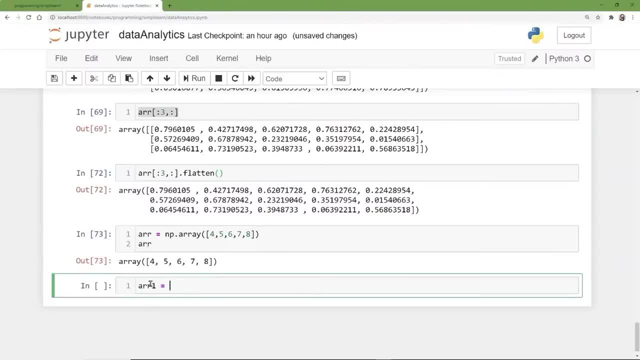 of reasons for that. One is runtime Because of the way the numpy array is set up. a lot of times you build your data and then push it into the numpy array instead of continually adding on to the array, And then it also usually it automatically generates a copy for protecting your data. 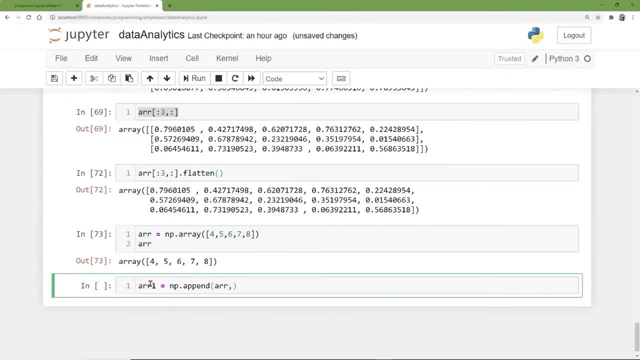 So there's a lot of reasons to be careful about appending this way, But you can certainly do it And we can just take our array. we're going to create a new array, array 1.. And if we print array 1 and we append 8 to it, you'll see 4, 5,, 6, 7, and then there's. 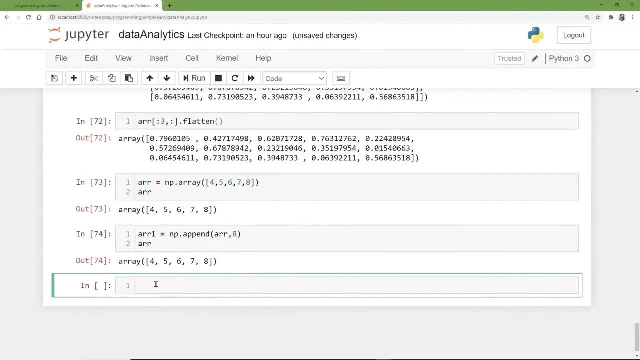 our 8 appended on to the end, And if you want to append something to an array, you'd probably also want to: oops, array 1.. Let's try that again. There we go. Now we have the 8 appended on to the end, so you can see 4,, 5,, 6,, 7,, 8, and then we 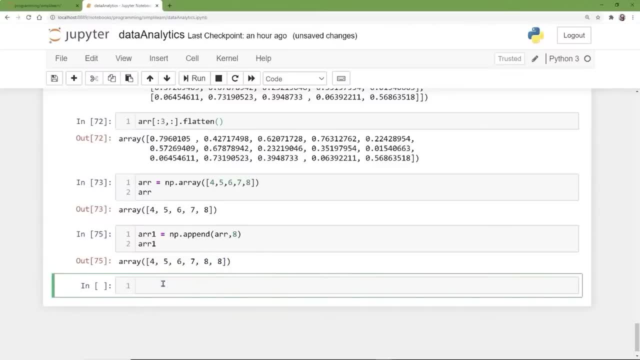 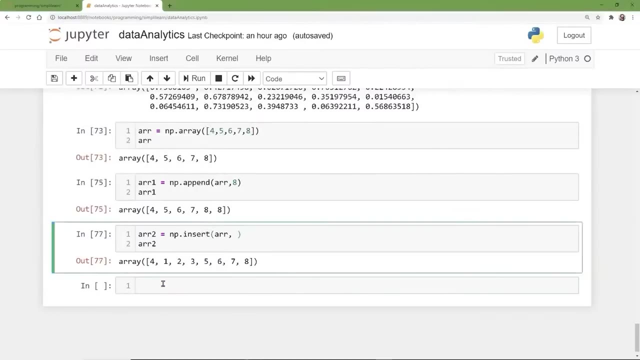 appended another 8.. 8 on there And if you're going to append something, you might want to go ahead and insert instead of appending. It might be you need to keep a certain order And we can do the same thing. We can do our array and we're going to append or insert at the beginning. 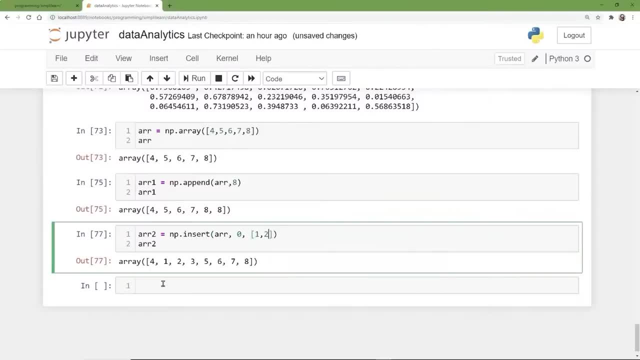 And let's go ahead and insert 1,, 2, 3,, 1,, 2, 3.. And we go ahead and print our array 2.. We run it and you can see 1,, 2,, 3 is inserted. 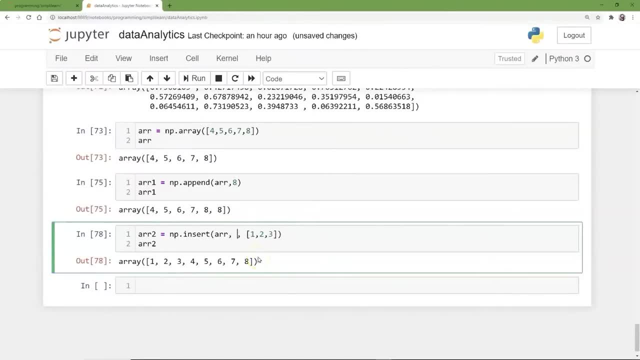 Insert is a lot more powerful in that you can put it anywhere in the array. We can move it to the 1 spot And there we go: 1,, 2,, 3.. We can do a minus 1, just for fun. 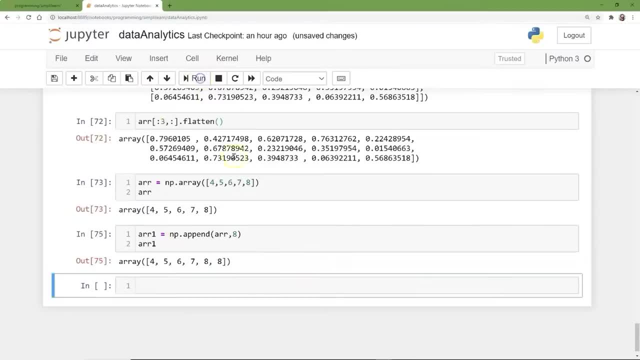 oops, array one. Let's try that again. There we go. Now we have the eight appended on to the end, So you can see four, five, six, seven, eight, and then we appended another eight on there. And if you're going to append something, 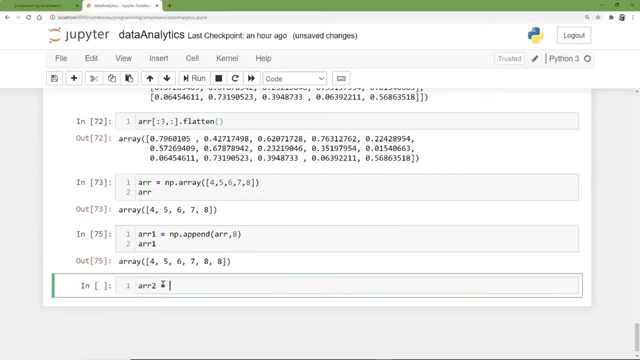 you might want to go ahead and insert Instead of appending. it might be. you need to keep a certain order And we can do the same thing. We can do our array and we're going to append or insert at the beginning. 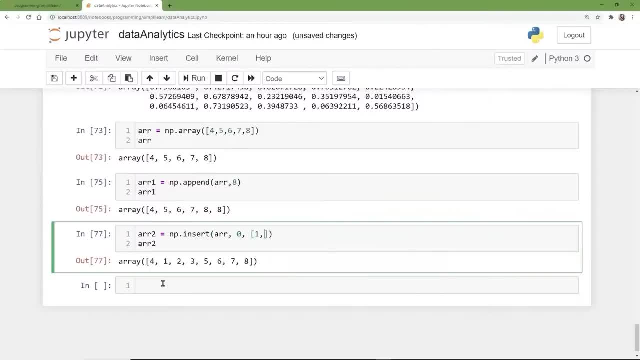 And let's go ahead and insert one, two, three, One, two, three, And we go ahead and print our array two. We run it and you can see one, two, three is inserted at the beginning. Insert's a lot more powerful. 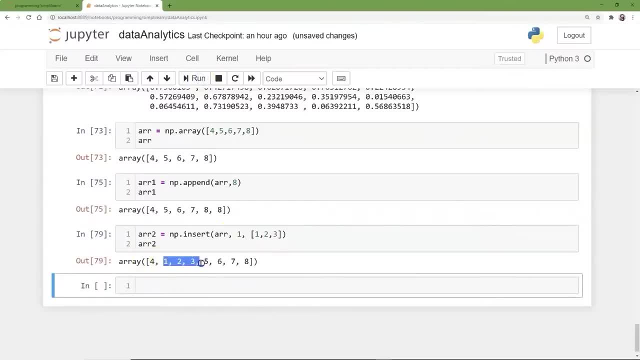 in that you can put it anywhere in the array, We can move it to the one spot And there we go. one, two, three. We can do a minus one just for fun, And you'll see it comes up one, two, three. 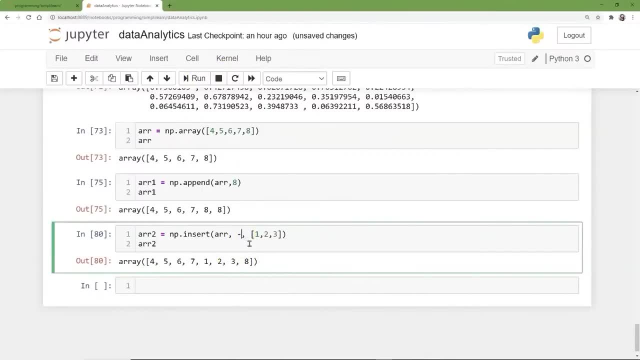 and we're counting backwards by one. I imagine you can do a minus zero And run this and it turns out that minus zero puts it back at the beginning, because that's how it registers a zero: It just takes a minus sign off. 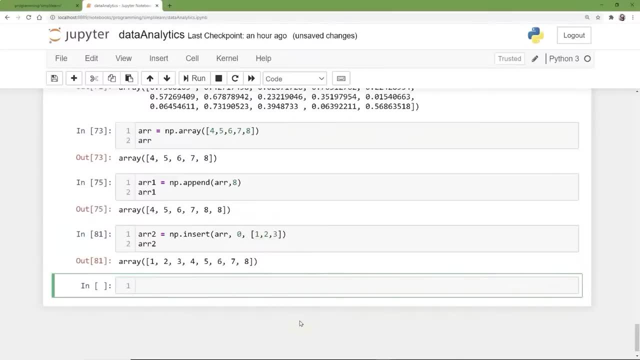 And just like we add numbers on, we might want to delete numbers, And so let's do an npdelete. Well, let's keep it a little bit, make it a little easy here to watch. We'll go ahead and create an array three. 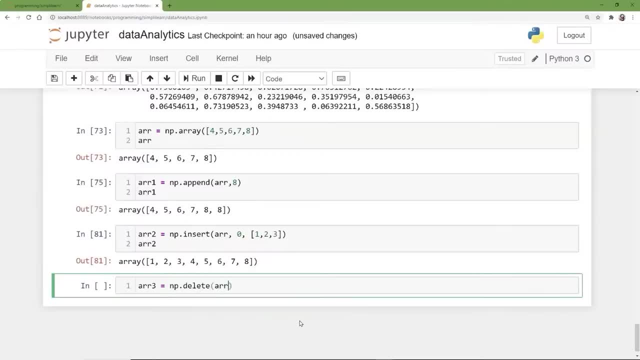 And we'll do npdelete. We were just working with array two And what we want to do is delete zero space. So if you look at this, here's our array two. Array two starts with one, And when we delete the space on here, 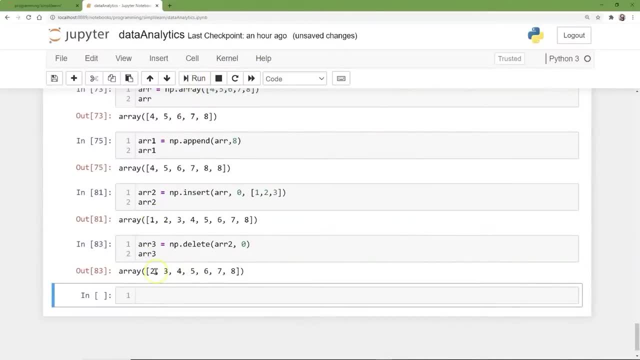 and print that out. we deleted the one right out of there. And we can also do something like this: where we can do it as a slice And we can do, let's do one comma three. And if we run one comma three, 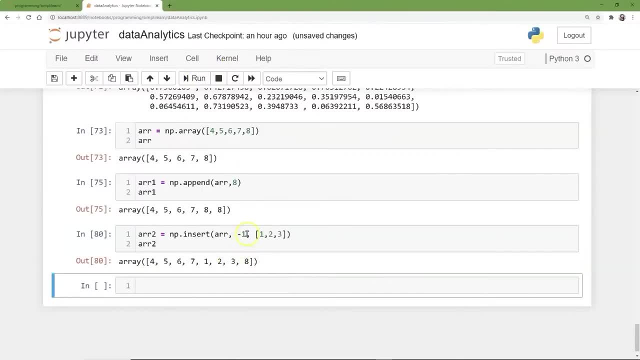 And you'll see it comes up 1,, 2,, 3, and we're counting backwards by 1.. I imagine you can do a minus 0 and run this And it turns out that minus 0 puts it back at the beginning, because that's how it registers. 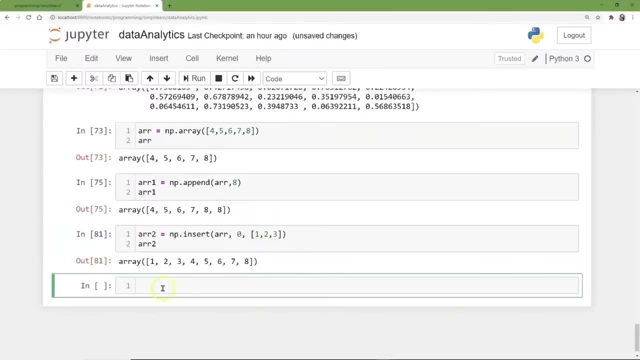 a 0. It just takes a minus sign off And just like that we're done. We're done. And just like we add numbers on, we might want to delete numbers, And so let's do an npdelete. Well, let's keep it a little bit, make it a little easy here to watch. 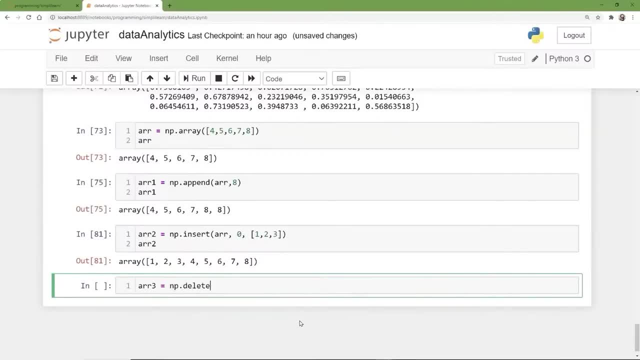 We'll go ahead and create an array 3. And we'll do npdelete. We were just working with array 2. And what we want to do is delete 0 space. So, if you look at this, here's our array 2.. 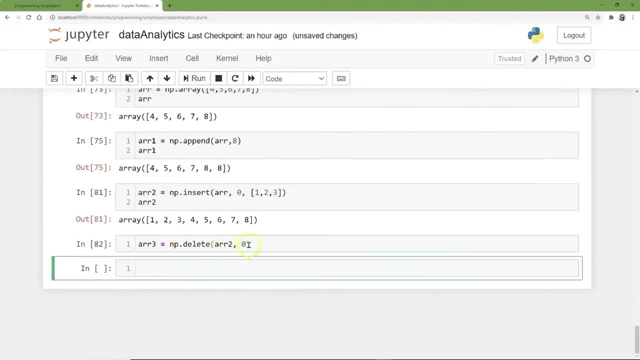 Array 2 starts with 1.. And when we delete the space on here And print that out, we've deleted the 1 right out of there. And we can also do something like this: where we can do it as a slice And we can do, let's do 1, 3.. 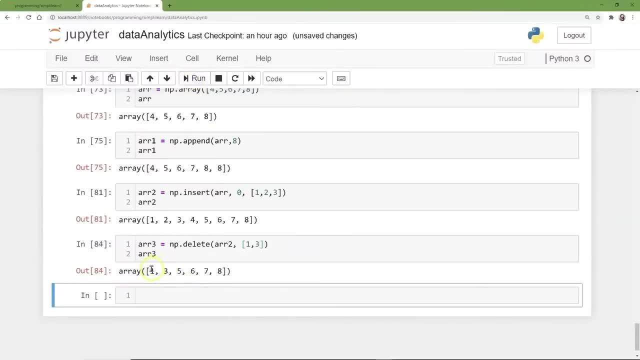 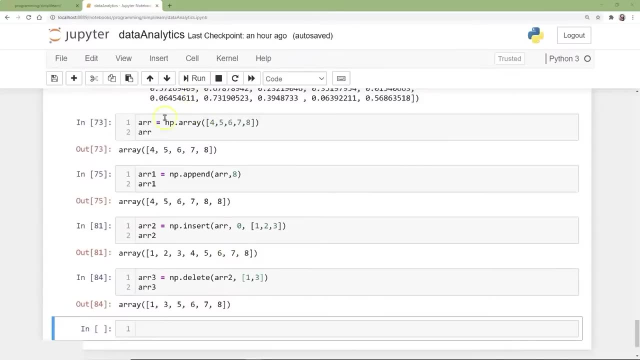 And if we run 1,, 3,, you'll see we've deleted the 1 space and the 3 space out, Which deleted our 2 and 4.. Now keep in mind when you're messing with adding lines and deleting lines. 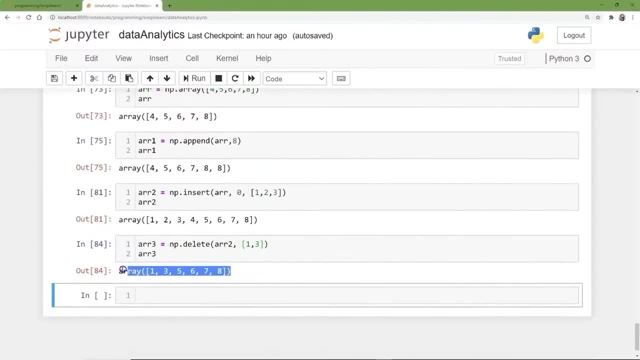 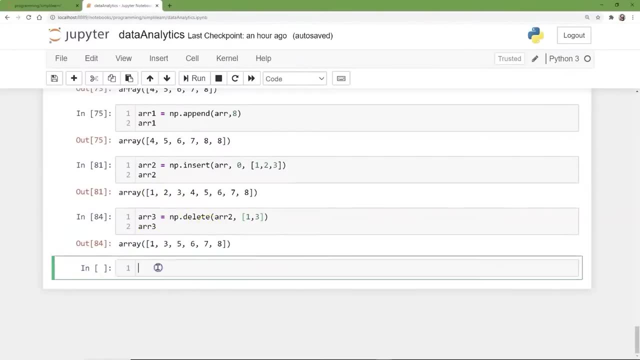 Uh, But you have to be really careful because there is a time element involved as far as where the data is coming from, and it's really easy to delete the wrong data and corrupt what you're working on or to insert stuff where you don't want it. 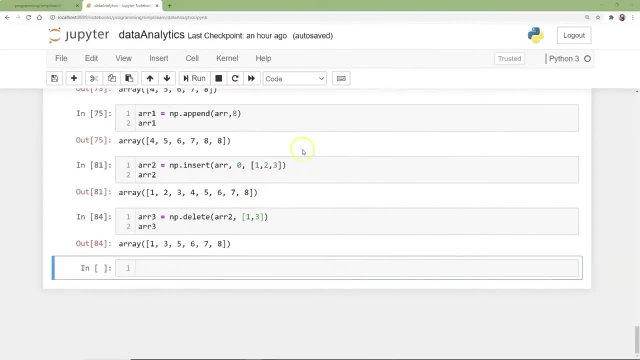 So there's always a warning when we talk about manipulating numpy arrays And, just like anything else we're doing, we'll create an array C, which equals- we'll just do our numpy array that we just created our numpy array 3, and we can do copy. 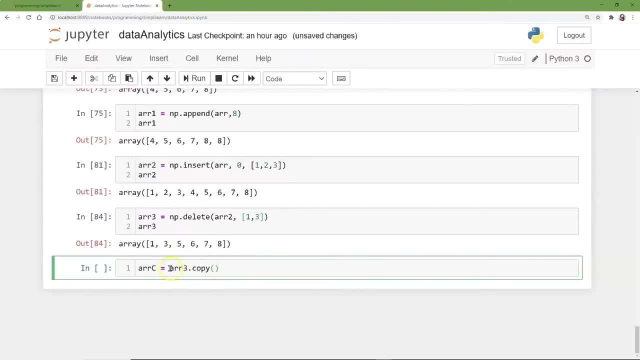 So you can make a copy of it. Maybe you want to protect your original data, or maybe you're making a mask and so you copy the array and then the new array, make all these alterations and change it from values to 0 to 1, to mask over the first one. 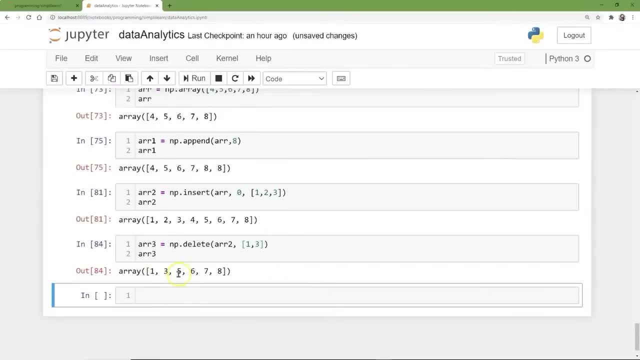 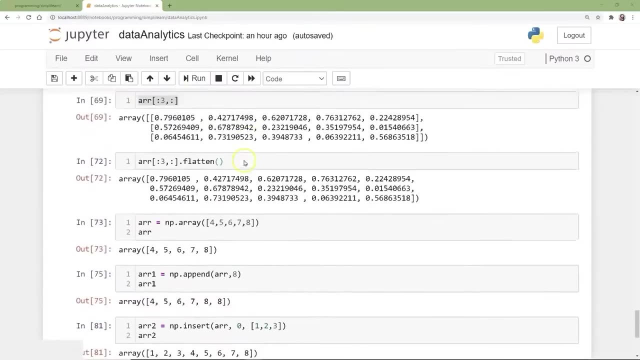 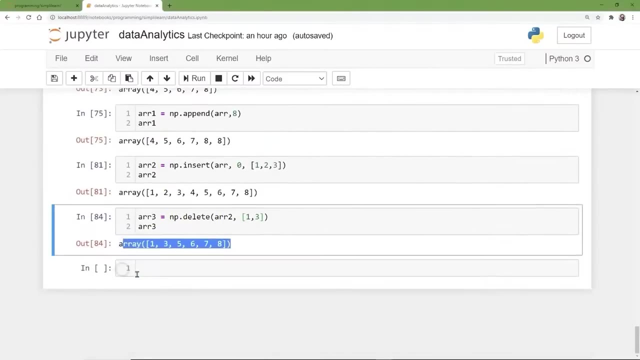 you'll see we've deleted the one space and the three space out, which deleted our two and four. Now keep in mind, when you're messing with adding lines and deleting lines, you have to be really careful because there's a time element involved. 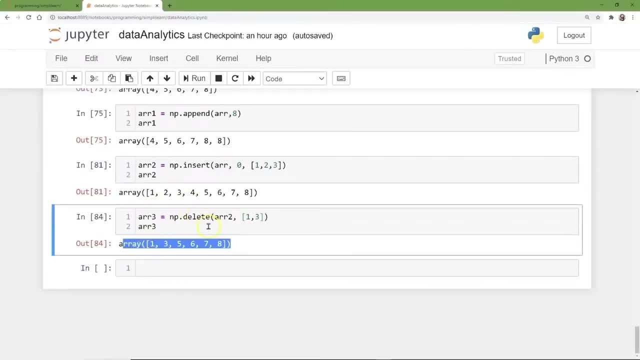 as far as where the data is coming from, And it's really easy to delete the wrong data and corrupt what you're working on or to insert stuff where you don't want it. So there's always a warning when we talk about manipulating numpy arrays. 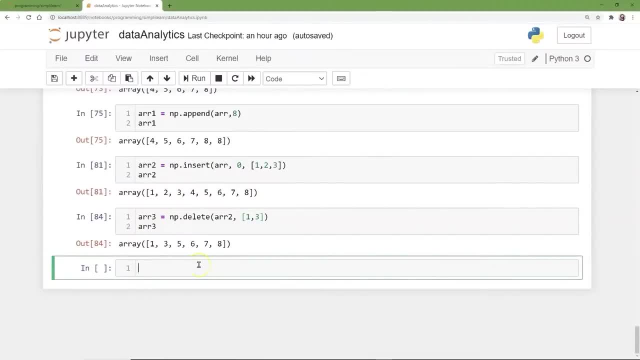 And, just like anything else we're doing, we'll create an array C which equals, we'll just do our numpy array that we just created our numpy array three And we can do copy, So you can make a copy of it. 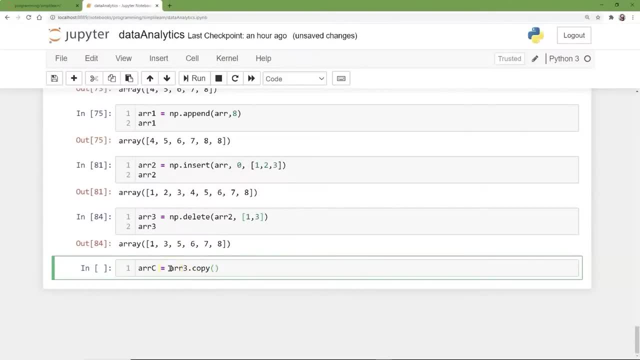 Maybe you want to protect your original data, or maybe you're making a mask, And so you copy the array and then the new array, make all these alterations and change it from values to zero, to one, to mask over the first one, And, of course, 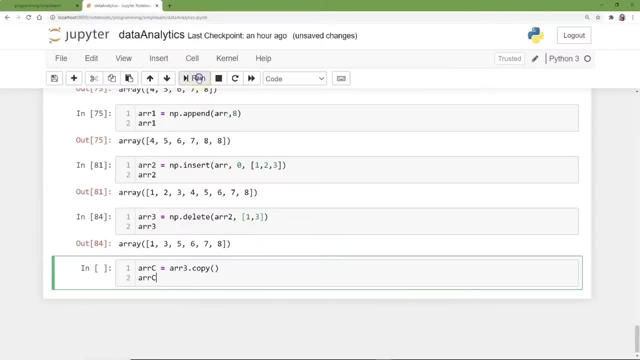 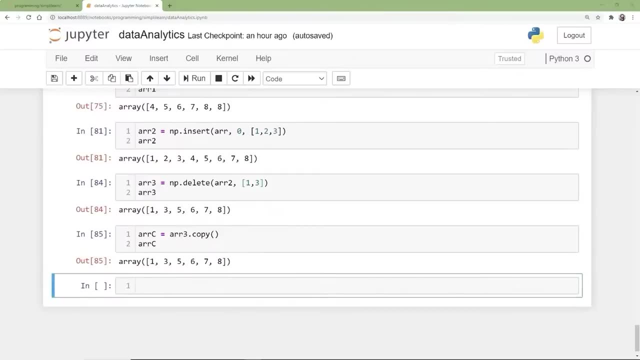 if we do array C, since it equals a copy of array three, it's the same thing: one, three, five, six, seven, eight. And now we're getting into combine and split arrays. I end up doing a lot of this. 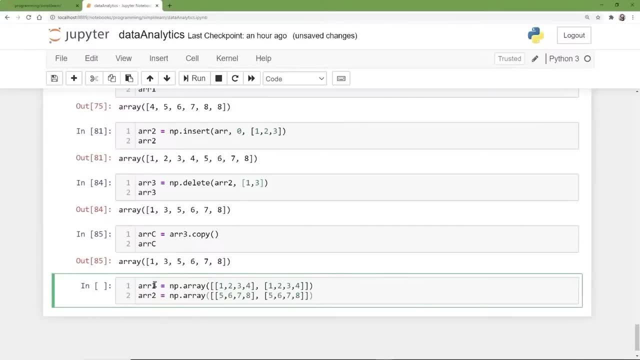 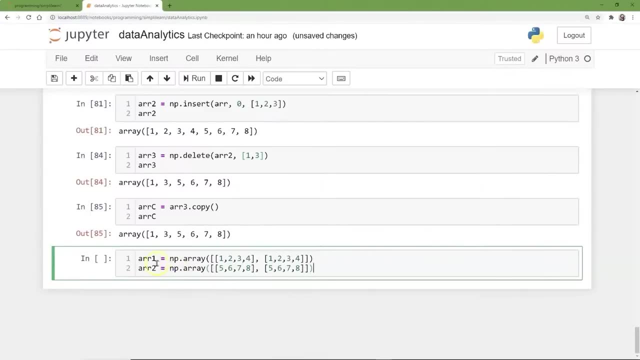 And I don't know how many times I end up fiddling with this and having a mess. So, but you do it a lot. You combine your arrays, you split them. you might need one set of data for one thing, another set of data for the other. 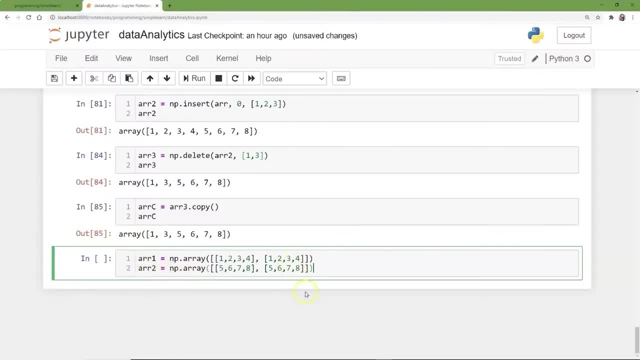 So let's go ahead and create two arrays: array one, array two- And I want you to note in the terminology we're going to look for is concatenate. What that means is we're going to take, we'll call this array cat. 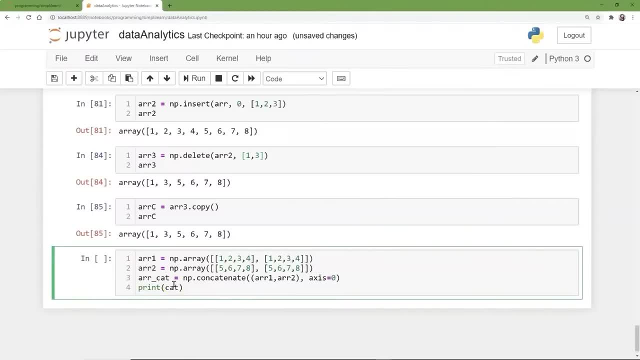 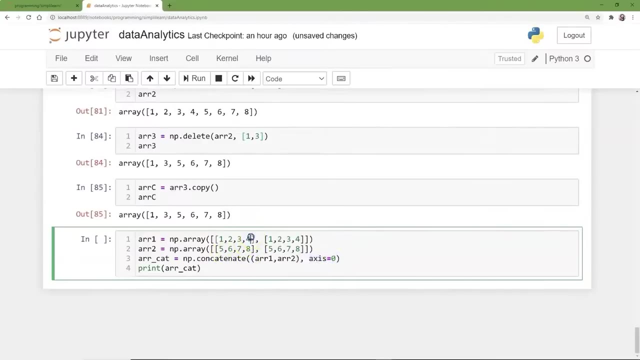 I like array cat. There we go, Our array cat, our concatenated array. we're taking array one and two and it's very important to really pay attention to your axes and your counts. I can't merge two arrays that have like if their axes are messed up. 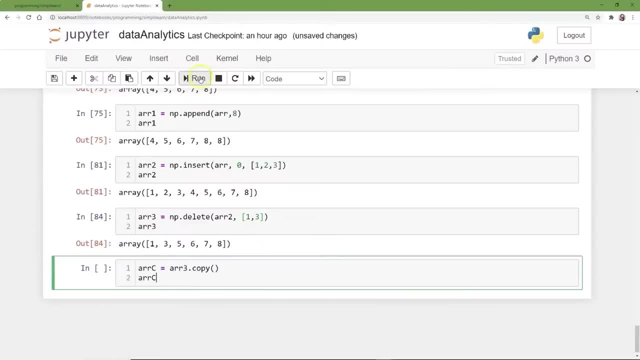 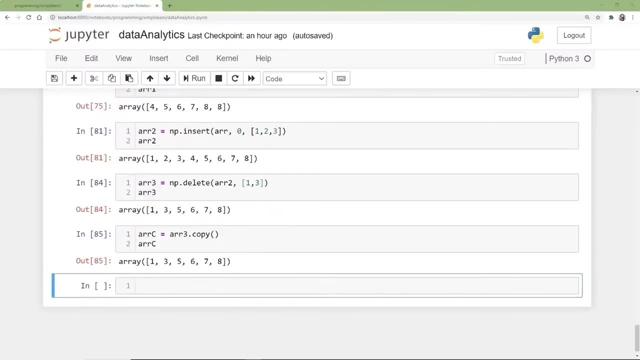 And, of course, if we do array C, since it equals a copy of array 3, it's the same thing: 1, 3,, 5, 6,, 7,, 8.. And now we're getting into combine and split arrays. 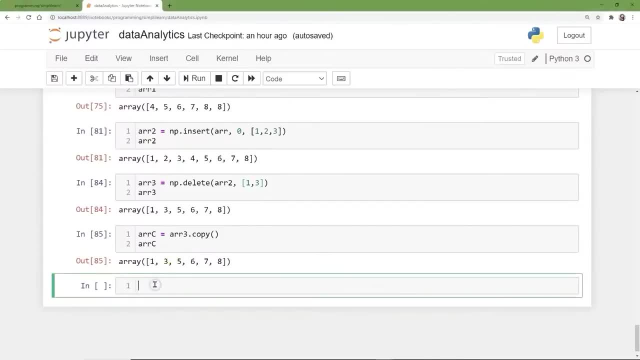 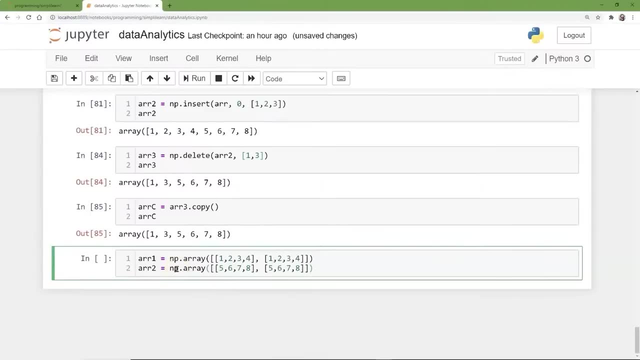 I end up doing a lot of this and I don't know how many times I end up fiddling with this and having a mess, But you do it a lot. You combine your arrays, you split them. you might need one set of data for one thing. 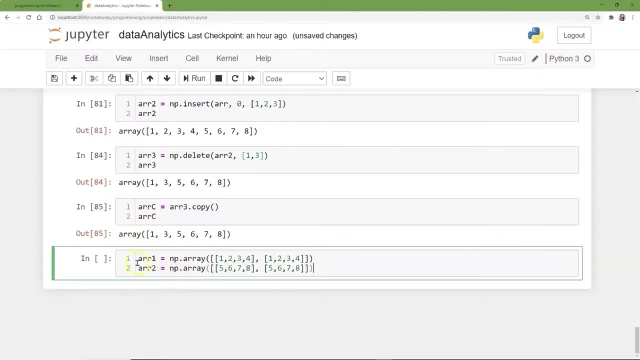 another set of data for the other. So let's go ahead and create two arrays, array 1, array 2.. And I want you to note, and the terminology we're going to look for is concatenating, And what that means is we're going to take, we'll call this array cat. 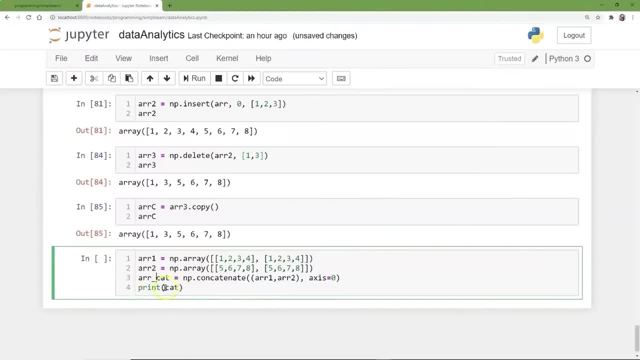 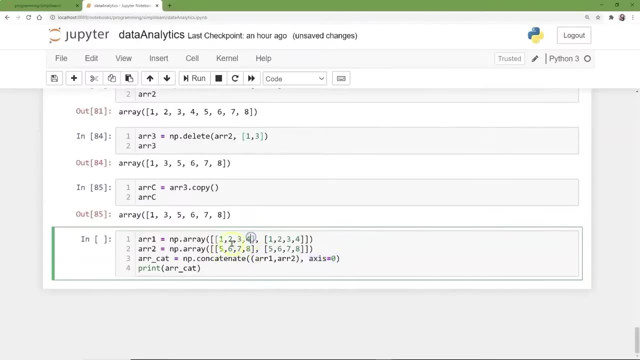 I like array cat. There we go, Our array cat, our concatenated array. we're taking array 1 and 2 and it's very important to really pay attention to your axes and your counts. I can't merge two arrays that have if their axes are messed up. and I'm merging on axis. 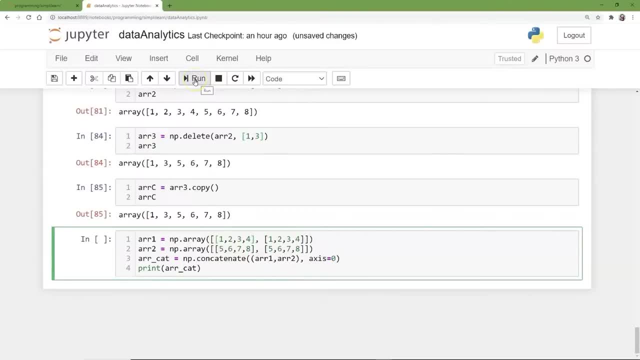 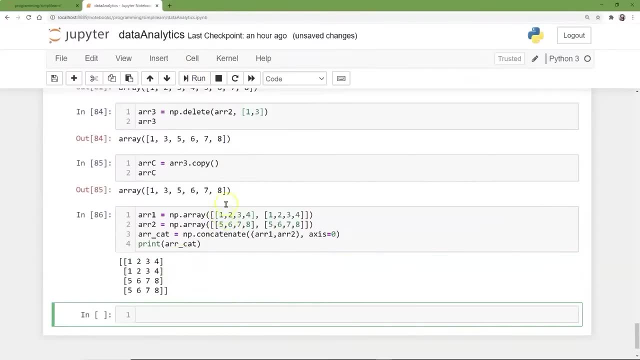 0. It's going to give me an error. I'm going to have to reshape them. So you got to make sure that whatever you're concatenating together works And what that means. as you can see, here we have 1,, 2,, 3, 4,. 1, 2,, 3, 4, and then 5,. 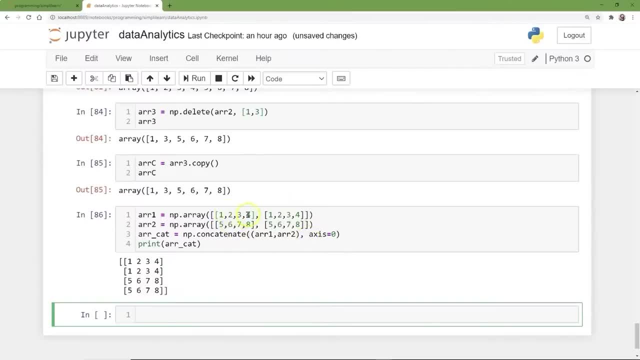 6,, 7,, 8,, 5,, 6,, 7,, 8 along the zero axes. These each are four values, So it's a two by four value, And if we go ahead and switch this to one, you can see how that flips it a little bit. 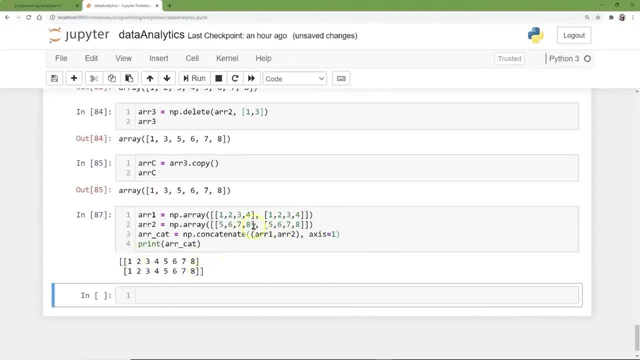 So now we have 1,, 2,, 3,, 4,, 5,, 6,, 7, 8.. It's interesting that we chose that, That one, if I did something like this where this is. now, there we go. 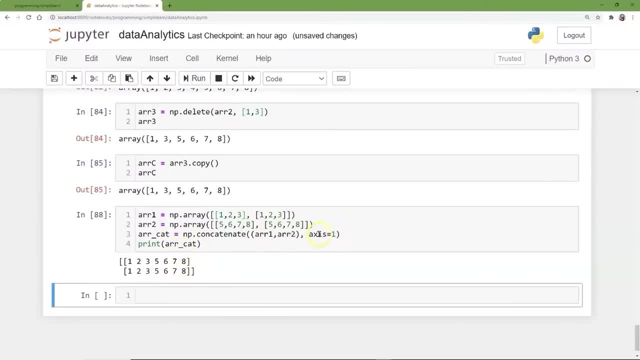 And we concatenate it, run this and it gives me an answer: okay, because I have two by two and I'm using axes one. But if I switch this to axes zero, where now it's got three and five, it gives me an error. 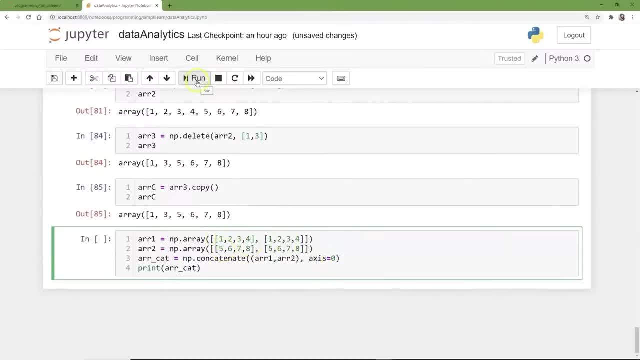 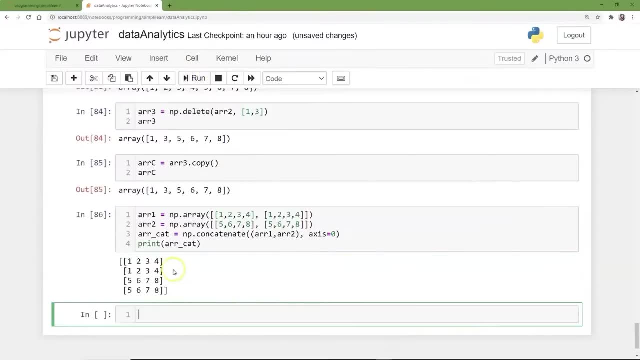 and I'm merging on axis zero. it's going to give me an error and I'll have to reshape them. So you got to make sure that whatever you're concatenating together works, And what that means. as you can see, here we have one, two, three, four. 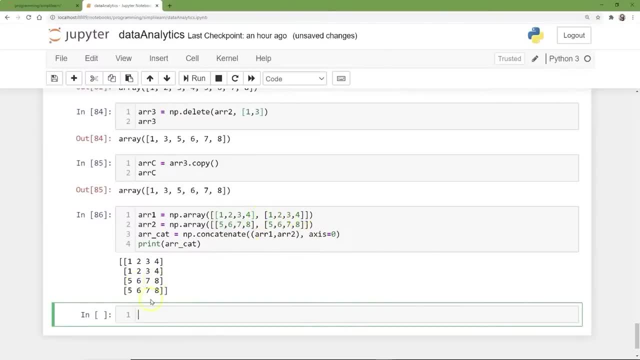 one, two, three, four and then five, six, seven, eight, five, six, seven, eight along the zero axes. These each are four values, So it's a two by four value, And if we go ahead and switch this to one, 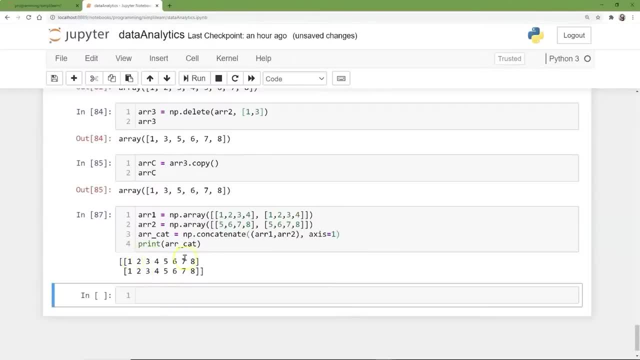 you can see how that flips it a little bit. So now we have one, two, three, four, five, six, seven, eight. It's interesting that we chose that one, If I did something like this, where this is now. 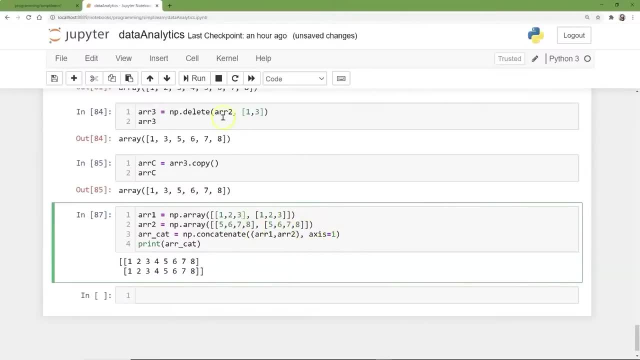 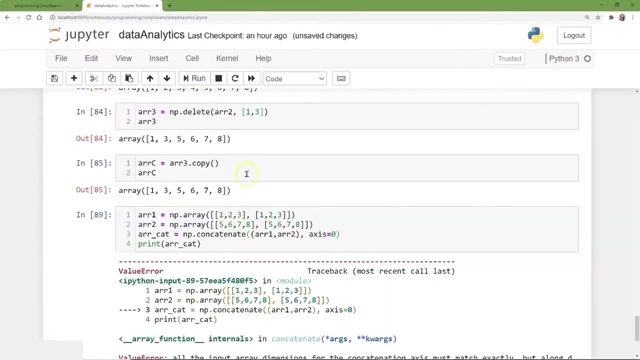 there we go and we concatenate it, run this and it gives me an answer: okay, because I have two by two and I'm using axes one. But if I switch this to axes zero, where now it's got three and five, it gives me an error. 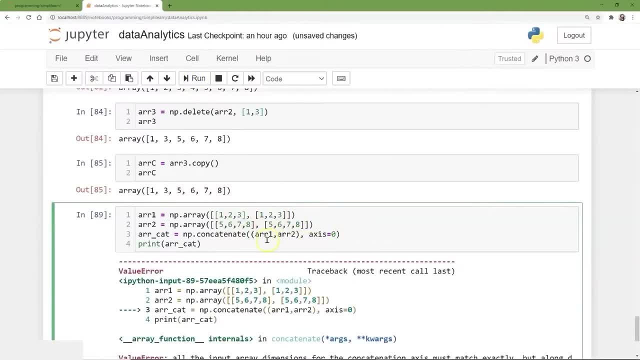 So you've got to be really careful on that to make sure that your whatever axes you are putting together, that they match. So, like I said, this one oops, axes one. axes one has two entities and since we're going on, axes one, 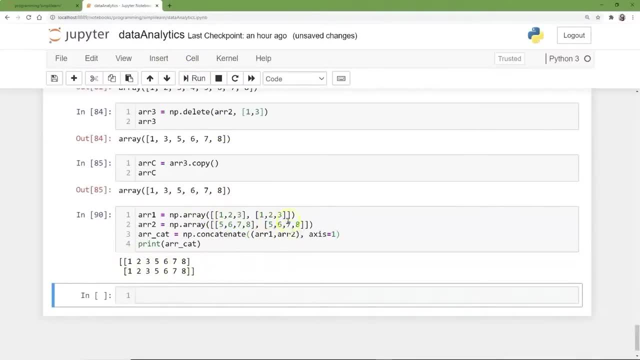 or by row. you can see that it lets it merge it right onto the end there, And you could imagine this if this was a xy plot of value, or the x value going in and the predicted y value coming out, and then you have another prediction. 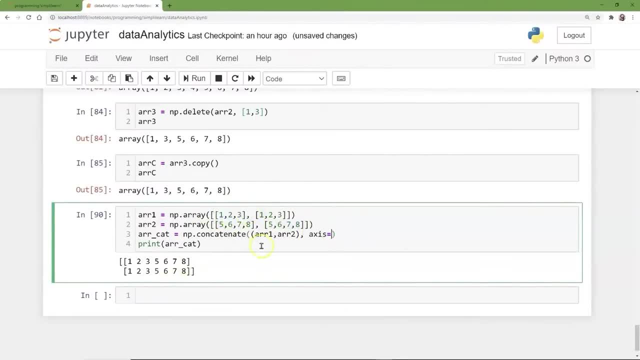 and you want to combine them. this works really easy for that, And we'll go back and let's just put this back to where we had it. Oops, I forgot how many changes I made. There we go, We'll just put it. 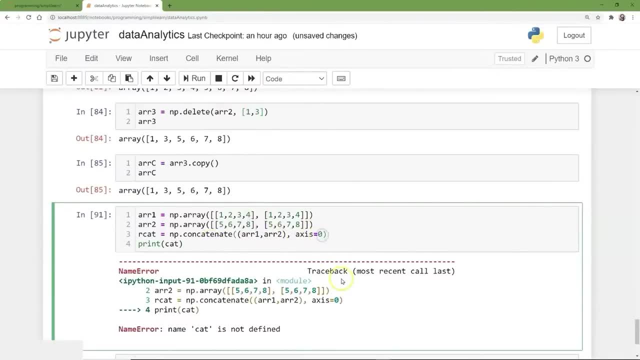 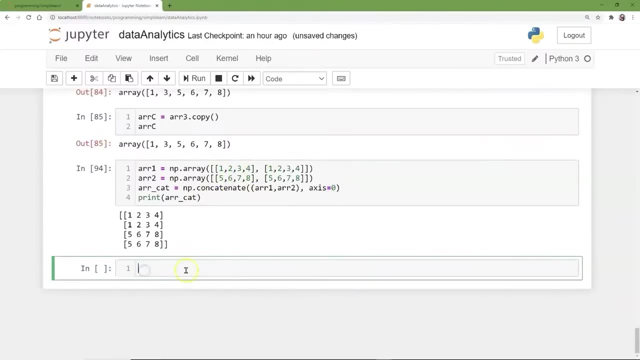 oops, I messed up on my concatenation order here. There we go. Okay, so you can see that we went through. the different concatenation Axes is really important when you're doing your concatenation values on here, And we'll switch this back to one. 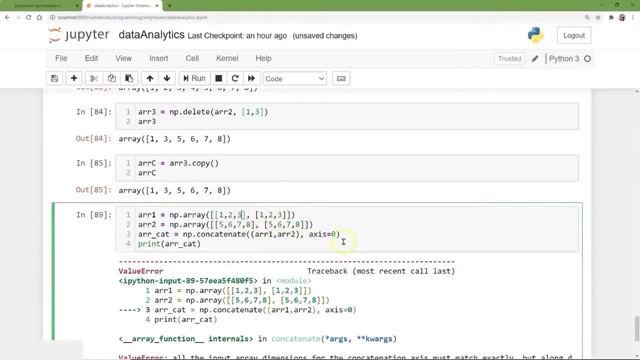 So you got to be really careful on that to make sure that your whatever axes you are putting together, that they match. So, like I said, this one, oops, axes one, Axes one has two entities and since we're going on axes one or by row, you can see that. 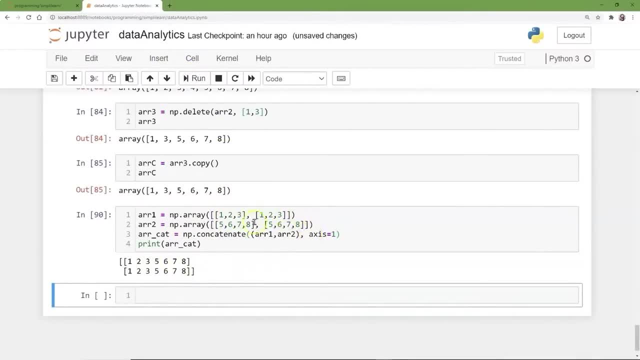 it, lets it merge it right onto the end there. And you could imagine this if this was a xy plot of value, or the x value going in and the predicted y value coming out, and then you have another prediction and you want to combine them. this works really easy for that. 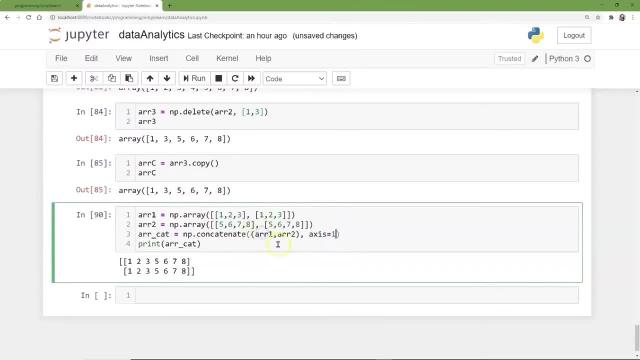 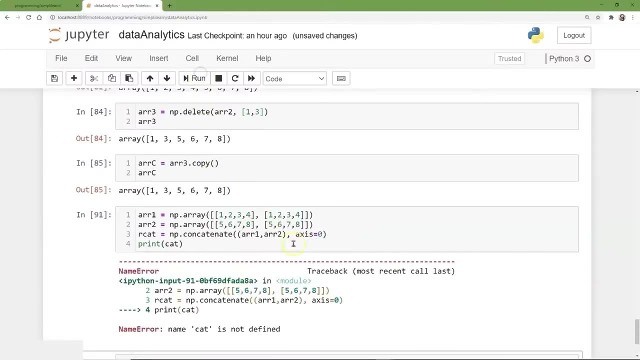 And we'll go back and let's just put this back to where we had it. Okay, Okay, Okay, Okay, Oops, I forgot how many changes I made. There we go, We'll just put it. oops, I messed up on my concatenation order here. 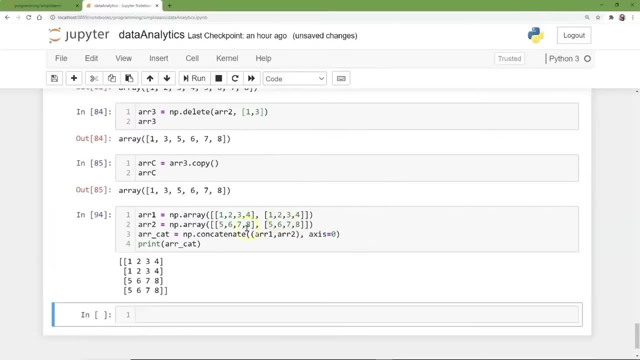 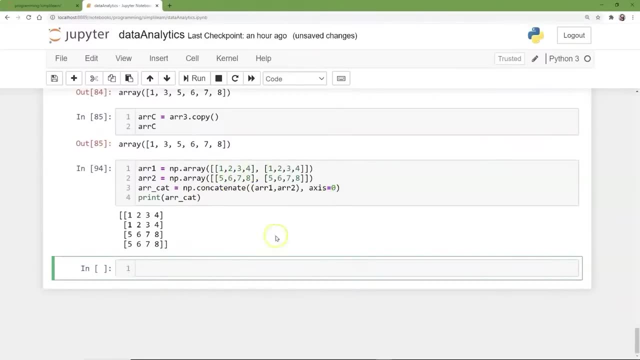 There we go. Okay, So you can see that we went through. the different concatenation Axes is really important when you're doing your concatenation values on here. We'll switch this back to one, just because I like the looks of that better. 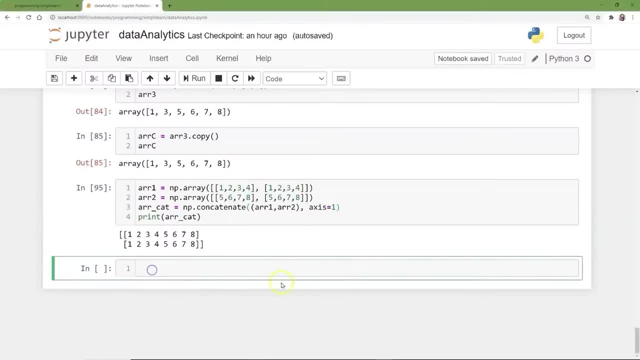 There we go Two rows. Now there are other commands in here, So we can do: cat v equals npvvstack. This is nothing more than your concatenation, but instead we don't have to put the axes in there, because v stands for vertical. 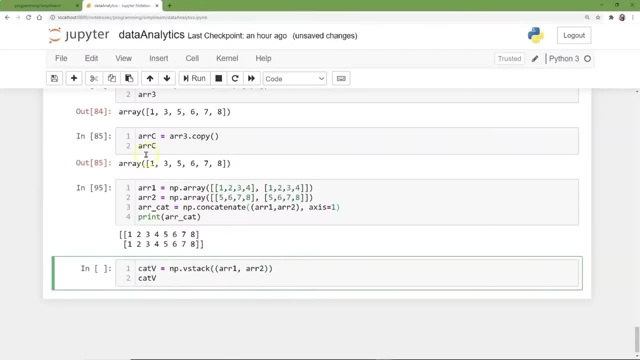 And so if we print out cat v and we run this, you can see we get the one, two, three, four. one two, three, four, five, six, seven, eight, nine, ten. Okay, So that's what we're looking for. 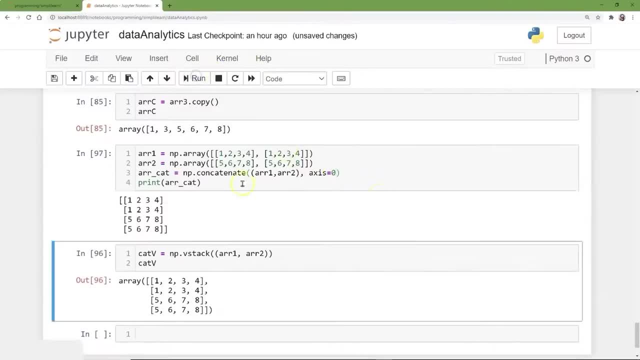 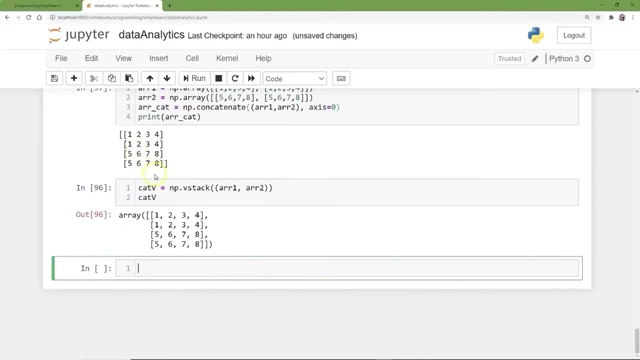 And that would be the same as making this axis zero for vertical stack. And if you're going to have a vertical stack, you can also have an h stack. So if we change this from v stack to oops, here we go h stack and we'll just change. 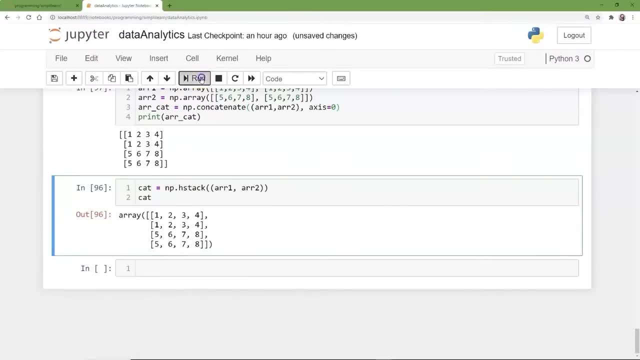 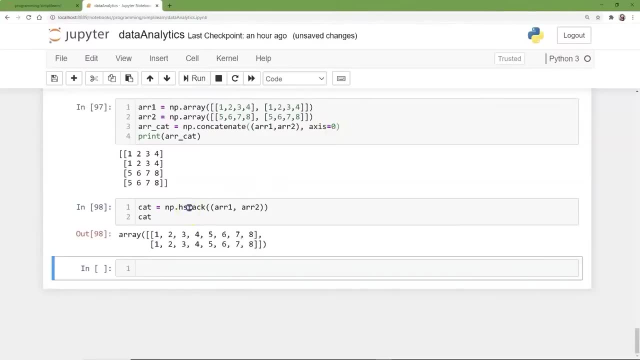 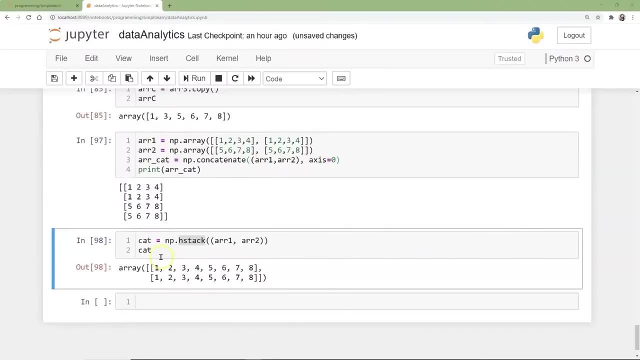 this from cat to cat and I run this. it's the same as doing axis zero. The process is identical in the background. This is like a legacy: setup Your v stack and your h stack. most people just use concatenate and then put the axes. 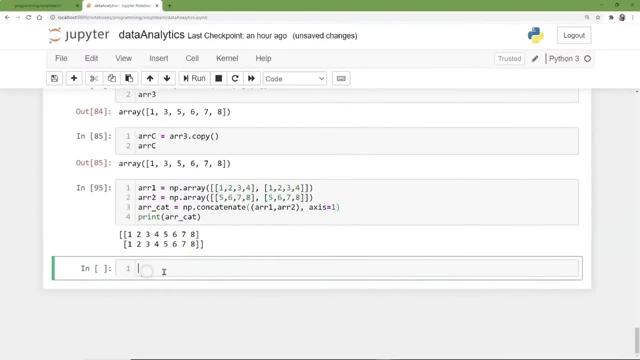 just because I like the looks of that better. There we go two rows. Now there are other commands in here, So we can do: cat v equals npvvstack. This is nothing more than your concatenation, but instead we don't have to put the axes in there. 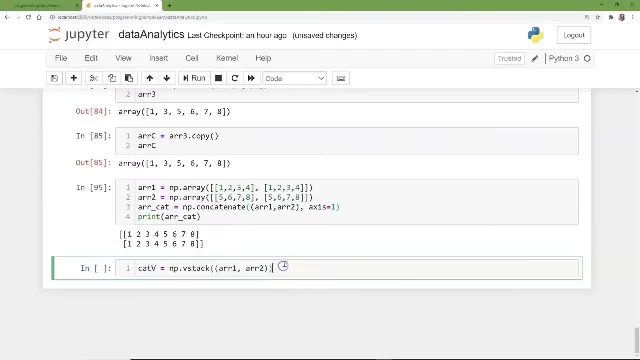 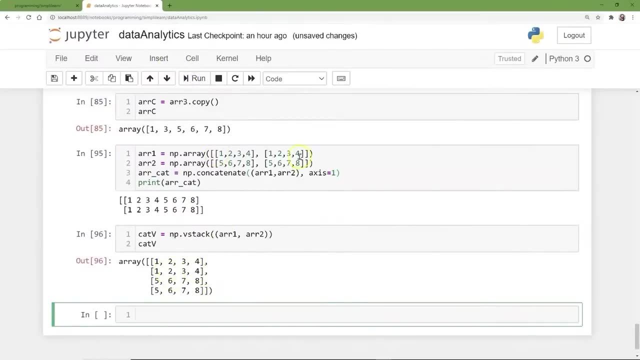 because v stands for vertical, And so if we print out cat v and we run this, you can see we get the one two, three, four. one two, three, four, and that would be the same as making this axis zero for vertical stack. 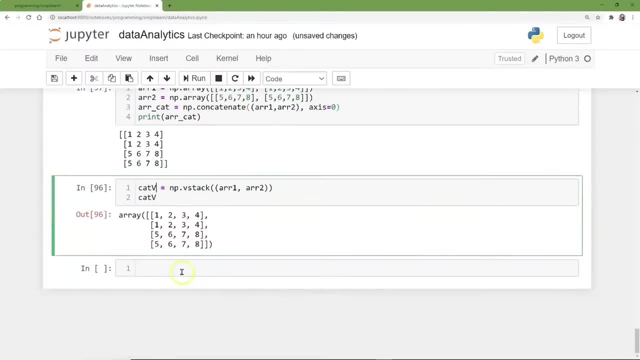 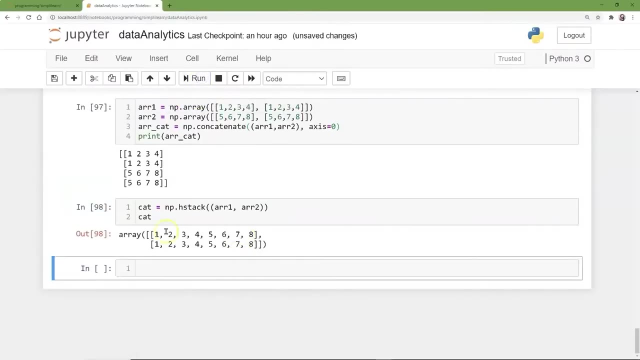 And if you're going to have a vertical stack, you can also have an hstack. So if we change this from vstack to oops, here we go hstack, and we'll just change this from cat to cat, and I run this. 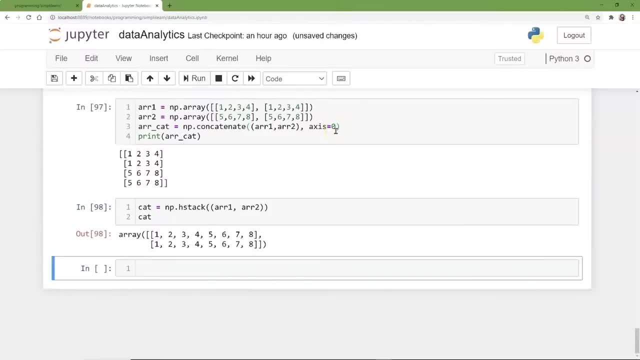 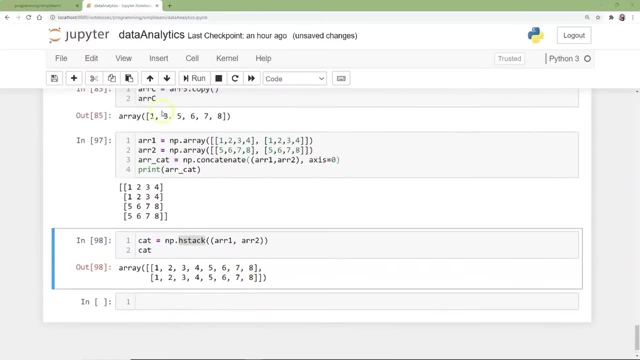 it's the same as doing axes zero. The process is identical in the background. This is like a legacy: setup your vstack and your hstack. Most people just use concatenate and then put the axes in there, because it has a lot more clarity. 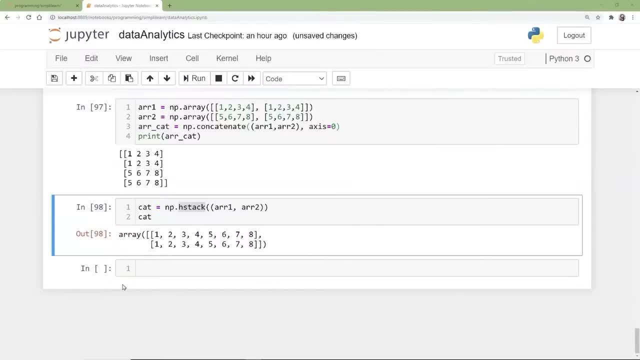 and is more commonly used nowadays. The last section in NumPy we're going to cover is kind of data exploration, And that'll make a little bit more sense in just a moment. Sometimes they call them set operations, But let's say we have an array. 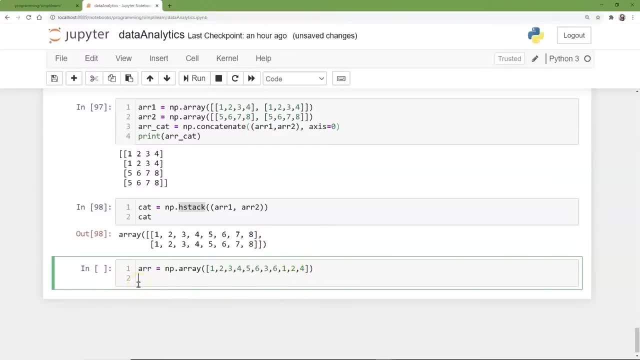 one, two, three, four, five, six, three, whatever it is. And so we generate an initial array here, And what I want to go ahead and do is find the unique values in that array, So maybe I'm generating what they call a one hot encoder. 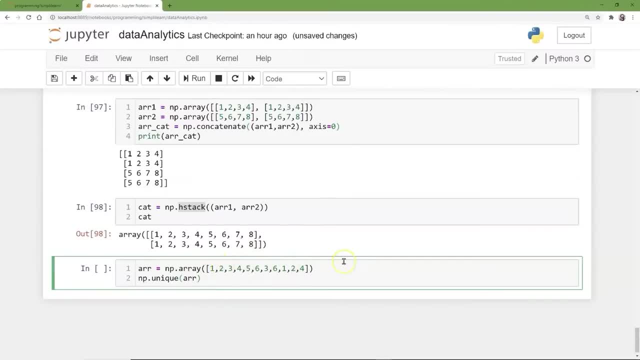 And so these values then all become. I need to know how long my bit array is going to be. So each word, how many? each word is represented by a number, And then I want to know just how many of those words are in there. 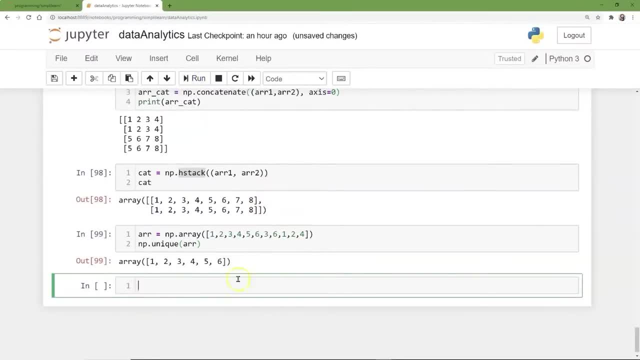 If we're doing word count- very popular thing to do- And you can see here when we do unique, we have one, two, three, four, five, six. Those are our unique values, Some of the things we can do with the unique values. 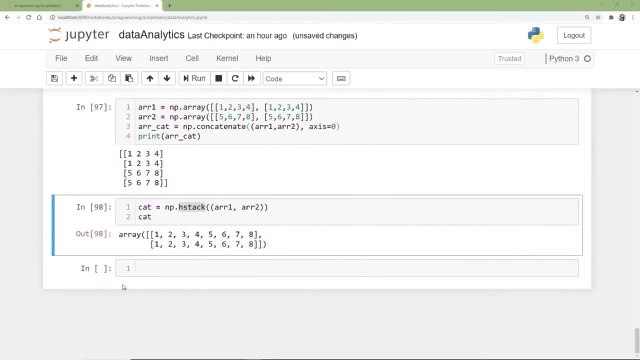 in there because it has a lot more clarity and is more commonly used nowadays. The last section in NumPy we're going to cover is kind of data exploration, and that'll make a little bit more sense in just a moment. Sometimes they call them set operations. 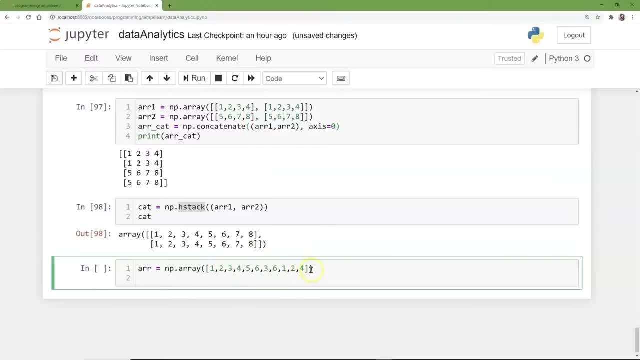 But let's say we have an array- One, two, three, four, five, six, seven, eight. So we have a set of three, four, five, six, three, whatever it is, And so we generate a nice little array here. 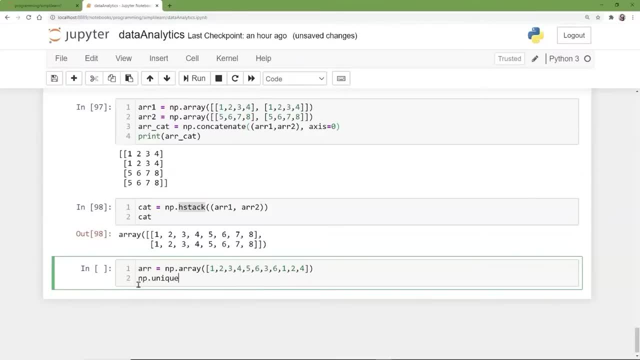 And what I want to go ahead and do is find the unique values in that array. So maybe I'm generating what they call a one hot encoder, And so these values then all become. I need to know how long my bit array is going to. 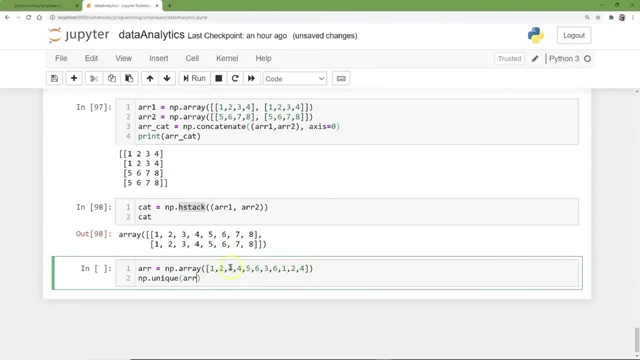 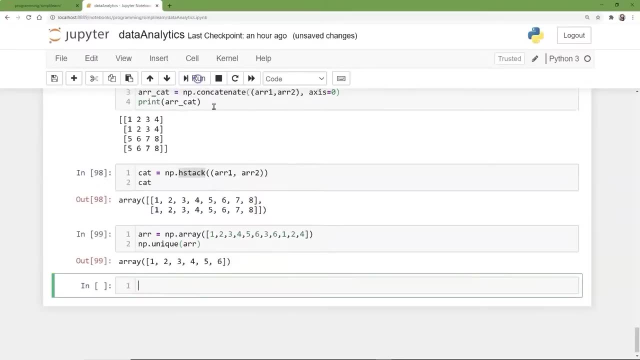 be. So each word, how many? each word is represented by a number, And then I want to know just how many of those words are in there. if we're doing word count- a very popular thing to do- And you can see here, when we do unique, we have one, two, three, four, five, six. 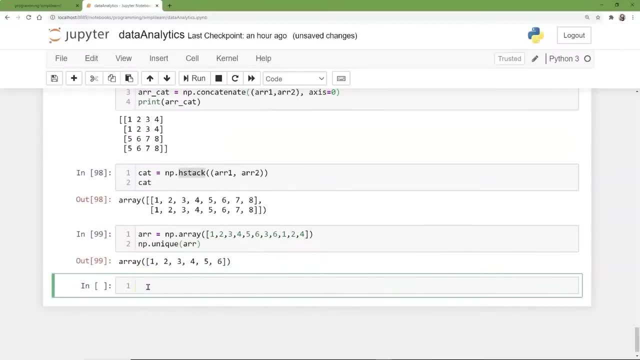 Those are our unique values. Some of the things we can do with the unique values is we can also, instead of doing just unique, we can do uniques, our unique values and counts of each unique value. And this is very similar to what we just did up here, where we were doing NP unique. but 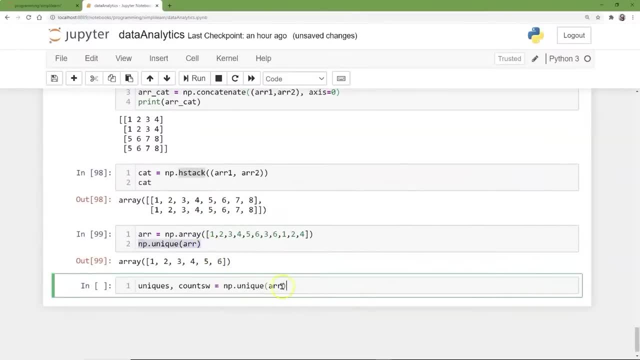 we're going to add a little bit more into there And it's just part of the argument. It's in this and we want to do: return counts equals, true. So instead of just returning the unique values, we want to know how many of those unique values. 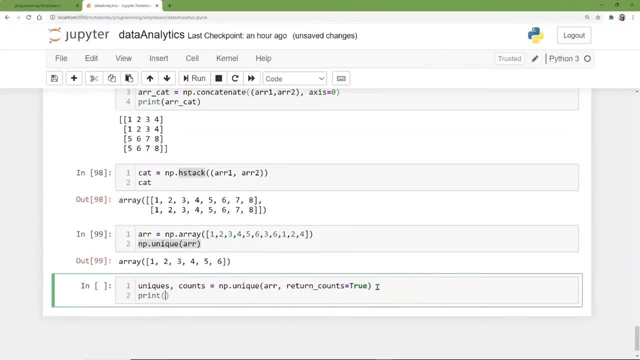 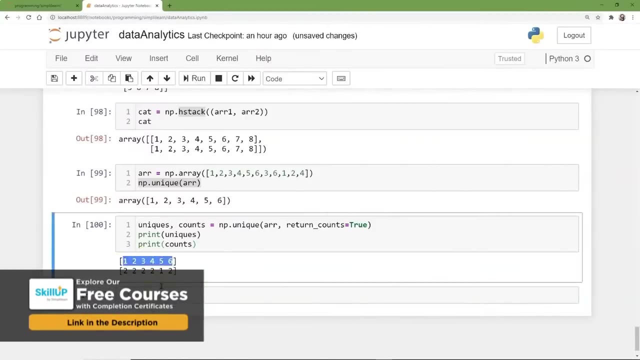 are in each one And we'll go ahead and print our uniques and print our counts When we run that. you can see here we have our unique value: one, two, three, four, five, six, just like we had before. 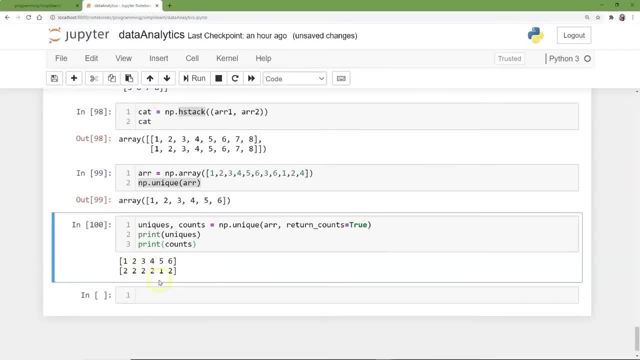 And then there's two of the first of two ones, two twos, two threes, two fours, one, five, two sixes and so on, And you can go through and actually look at that if you want to count them. 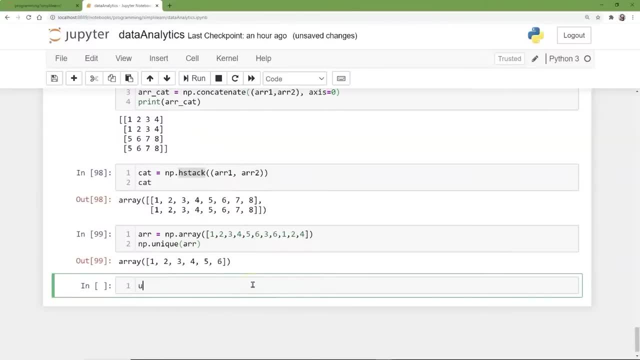 is. we can also, instead of doing just unique, we can do uniques, Our unique values and counts of each unique value. And this is very similar to what we just did up here, where we were doing np unique, But we're going to add a little bit more into there. 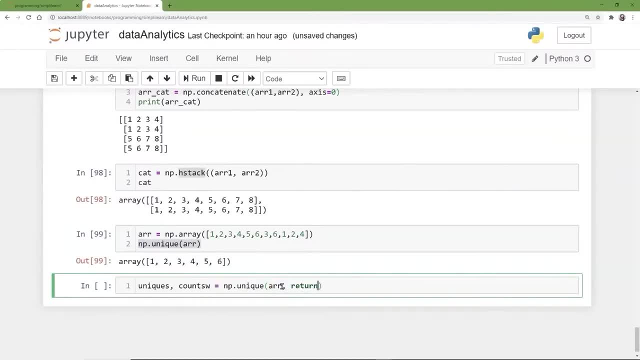 And it's just part of the arguments in this, And we want to do return counts equals, true. So instead of just returning the unique values, we want to know how many of those unique values are in each one, And we'll go ahead and print. 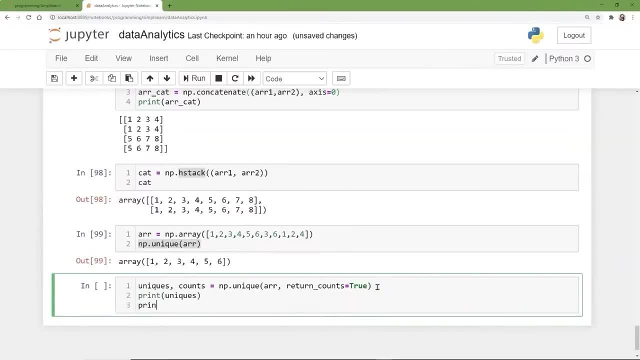 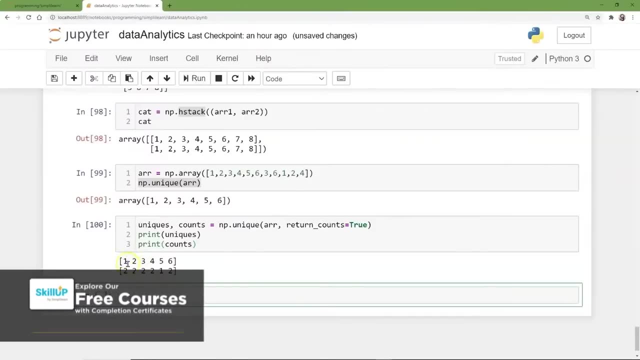 Our uniques And print Our counts When we run. that you can see. here we have our unique value: one, two, three, four, five, six, Just like we had before. And then there's two of the first of two ones. 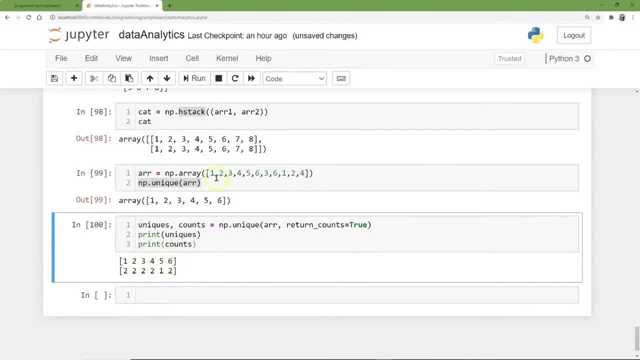 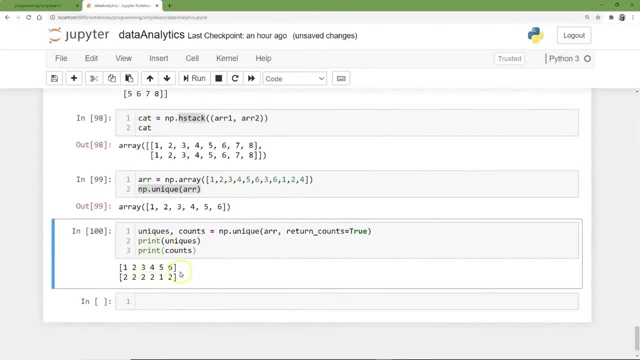 two twos, two threes, two fours, one five, two sixes and so on, And you can go through and actually look at that if you want to count them. But a quick way to find out your distribution of different values. 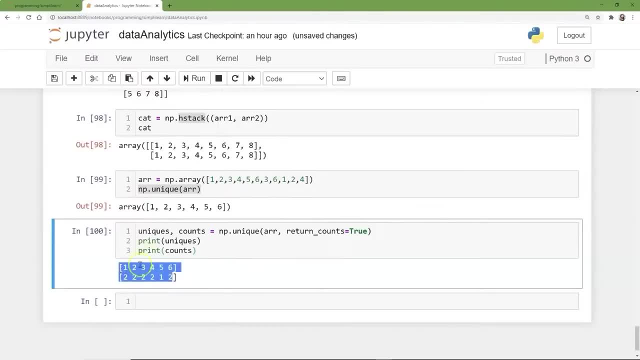 You want to know how often the word the is used versus the word and If each word is represented as a unique number And along the set variables we might want to know. let me just put a note up here We're going to start looking at. 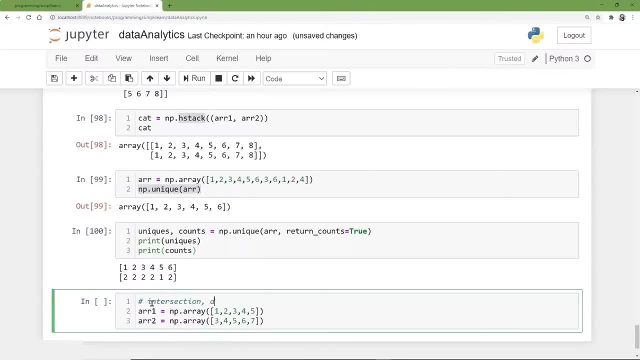 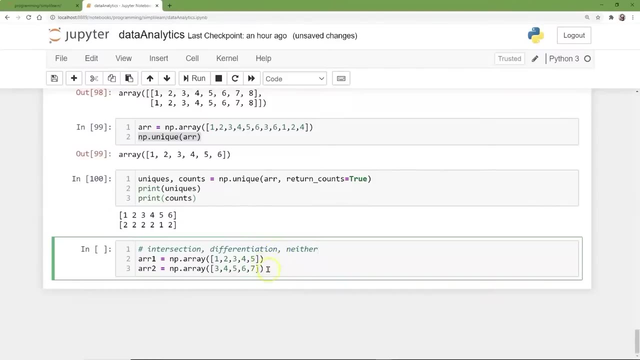 intersection, And we might want to also know differentiation, And neither. So when we're whoops neighbor, Neither. So what we're looking at now is we want to know: hey, where do these two arrays intersect? And we have one, two, three, four, five. 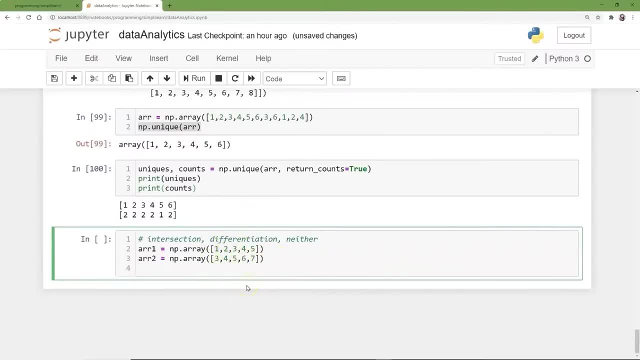 three, four, five, six, seven. We might want to know what is common between the two arrays. And so when we do that, we have NP intersect And it's a one D array, one dimensional array, And then we need to go ahead and put. 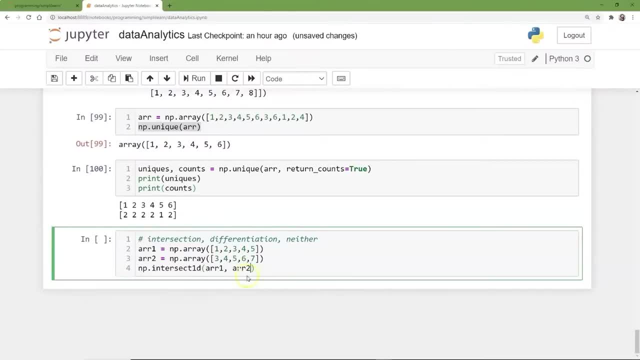 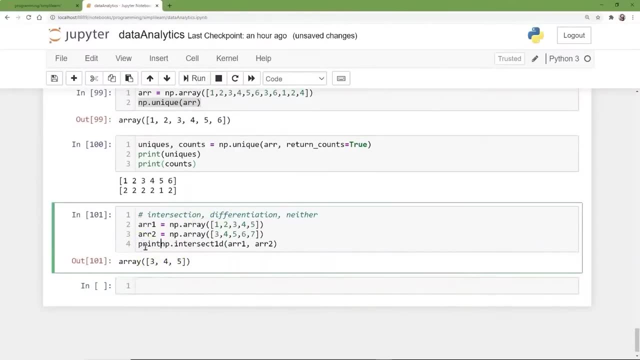 array one, array two And if we run this we can see they intersect at three, four, five. That's what they have common And because we're going to go ahead and go through these and look at a couple different options, 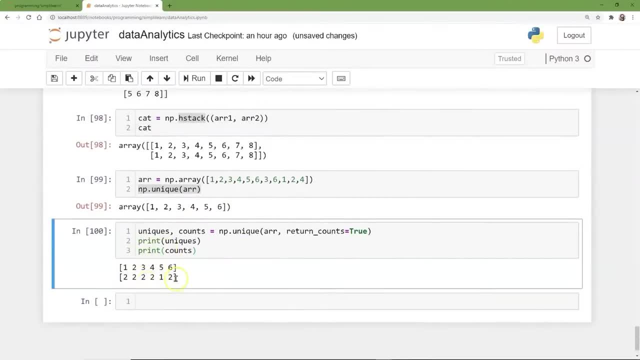 But a quick way to find out your distribution of different values. So you might want to know how often the word- the- is used versus the word and if each word is represented as a unique number And along the set variables we might want to know. 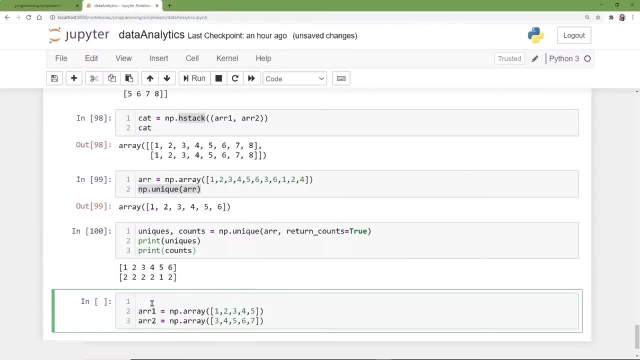 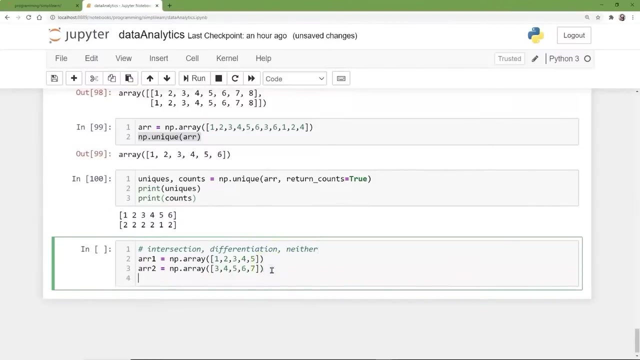 Let me just put in here, Let me just put a note up here. We're going to start looking at intersection And we might want to also know differentiation and neither. So when we're whoops, neighbor, neither. So what we're looking at now is we want to know: hey, where do these two arrays intersect? 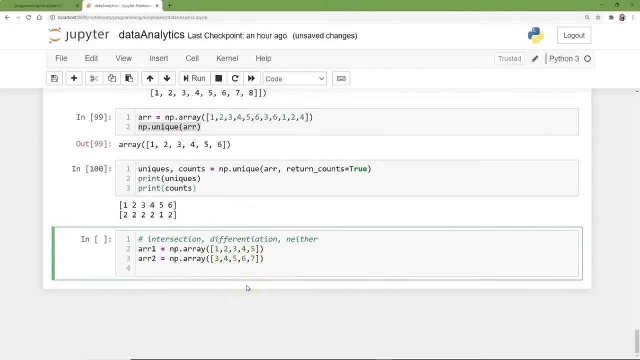 And we have one, two, three, four, five, three, four, five, six, seven. We might want to know what is common between the two arrays. And so when we do that, we have NP intersect and it's a 1D array, one-dimensional array. 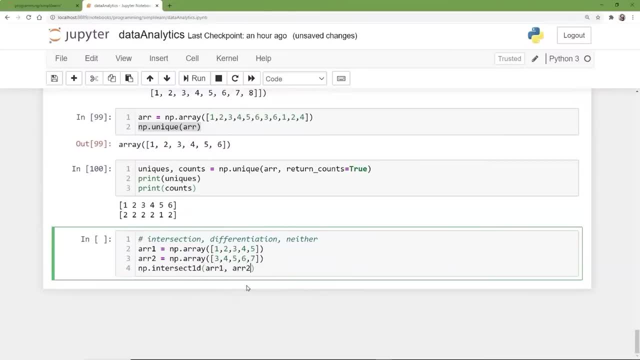 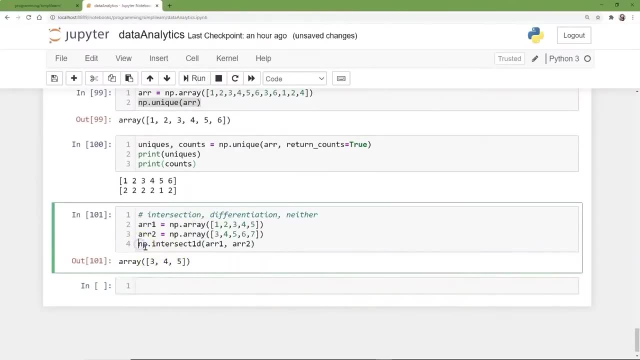 And then we need to go ahead and put array one, array two And if we run this we can see they intersect at three, four, five. That's what they have common. I'm being careful, All right, All right. 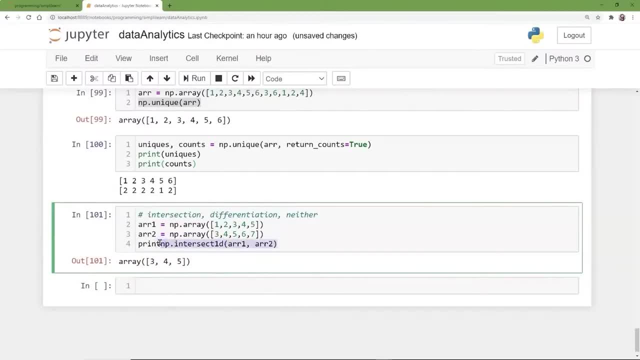 All right. So because we're going to go ahead and go through these and look at a couple different options, let's change this from intersect 1D and we'll do the same thing. We'll go ahead and print this So we might want to know the intersection where they have commonalities. 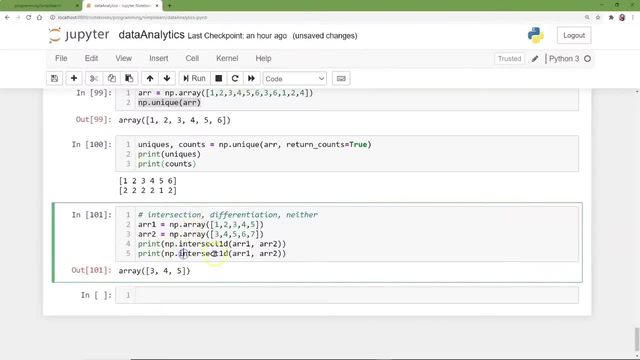 Another unique word is union of 1D. So instead of intersect, we want to know all the values that are in both of them. So here's our union of 1D, and when we run that you can see we have one, two, three. 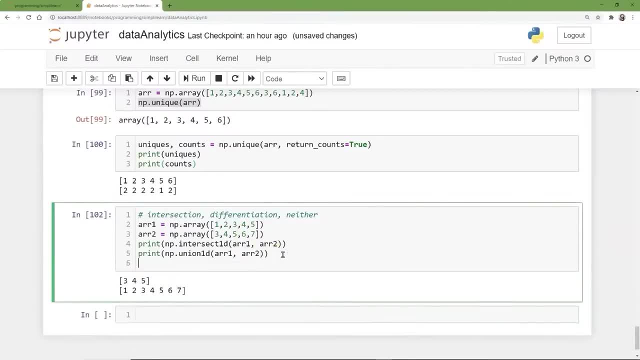 four, five, six, seven. So that's all the different values in there, And one of the last words- we have two more to go- is we want to know what the set difference is. So that's where you'll see. if you remember set- we talked about that being what they call these things- 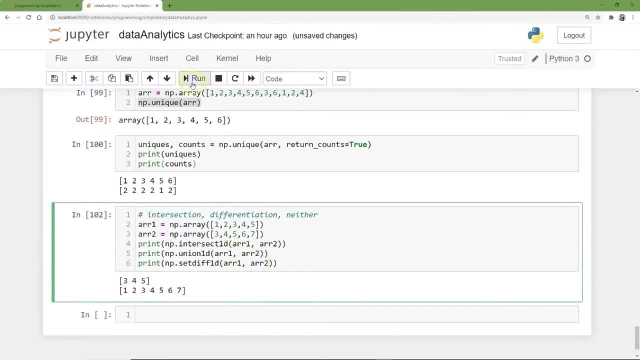 So the set difference of a 1D array. when we run that you can see that one is only in one array and two is only in one array. And if we want to know what's in array 1, but not in array 2, we might want to know what is in array 1, but not 2,. 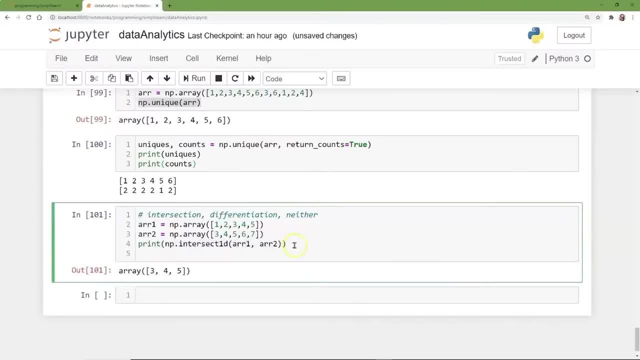 let's change this from intersect one D And we'll do the same thing. We'll go ahead and print this, So we might want to know the intersection where they have commonalities. Another unique word is union of one D, So instead of intersect. 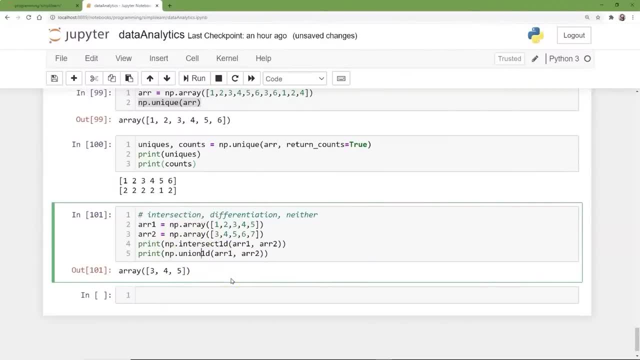 we want to know all the values that are in both of them. So here's our union of one D. When we run that you can see we have one, two, three, four, five, six, seven. So that's all the different values in there. 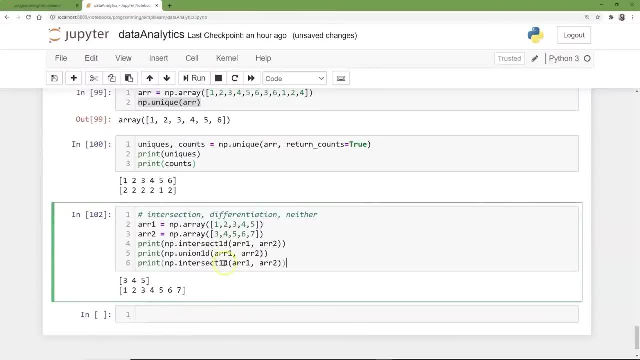 And the last, one of the last words- we have two more to go- is we want to know what the set difference is, And so that's where the you'll see. if you remember, set- we talked about that being what they call these things. 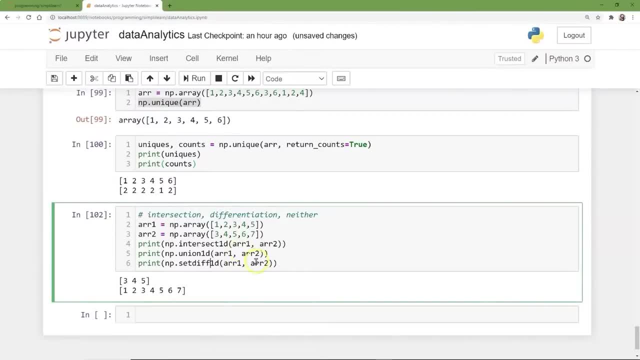 So the set difference of a one D array. when we run that you can see that one is only in one array and two is only in one array. And if we want to know what's in array one but not in array two, 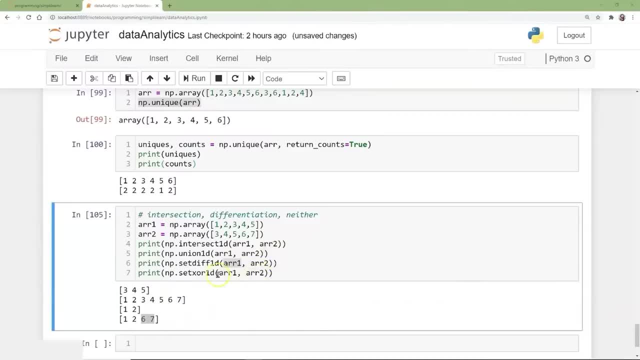 we might want to know what is in array one but not two, and what's in two but not one, And this would be the set X or one D on here. So we have the four different options here where we can do an intersection. What do they both have in common? 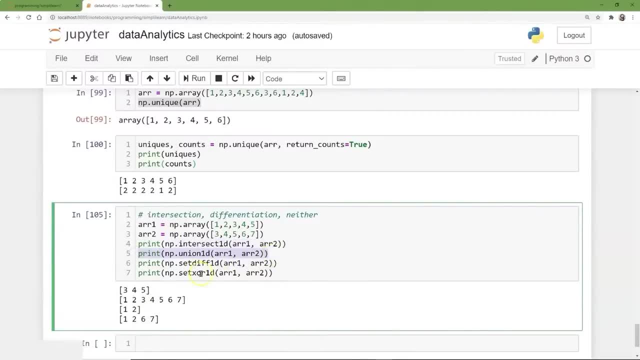 We can do a union. What are all the unique values in both arrays? We can see the difference: what's in array one but not array two. So set diff one, D, And then set X or what is not in one but is in two. 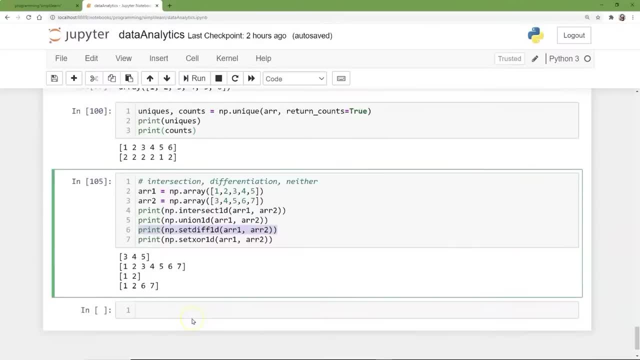 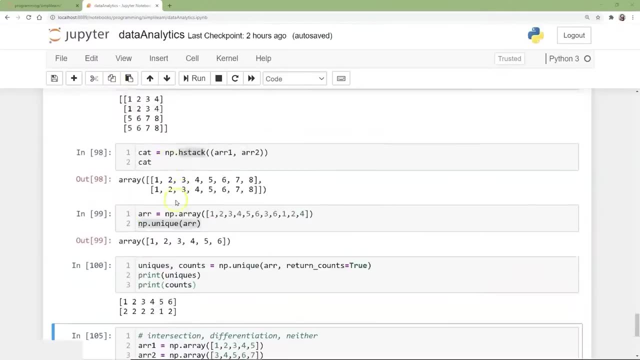 and what is not in two but in one. So we dug a lot in NumPy because we were talking. there's a lot of different little mathematical things going on in NumPy. A lot of this can also be done in pandas, although usually the heavy lifting is left for NumPy. 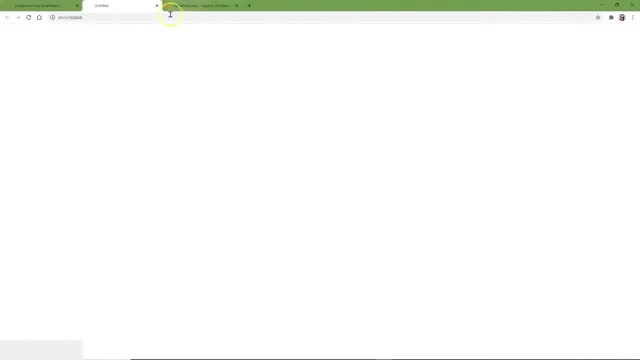 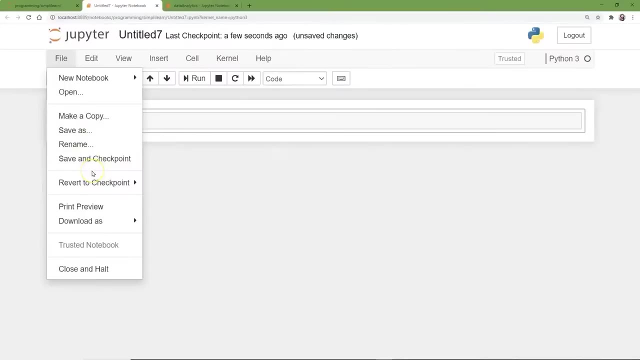 because that's what it's designed for. Let's go ahead and open up another Python 3 setup in here, And so we want to explore what happens when you want to display this. This is where it starts getting, in my opinion, a little fun. 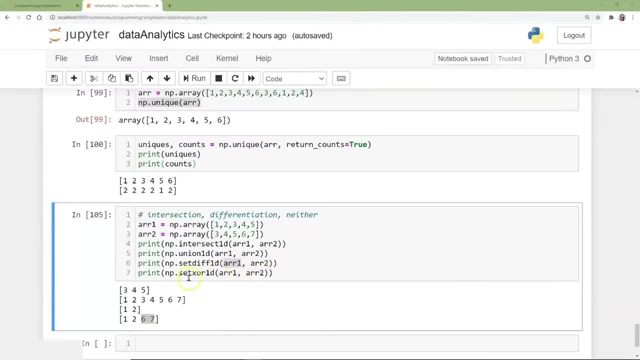 and what's in 2, but not 1, and this would be the set XOR 1D on here. So we have the four different options here where we can do an intersection. what do they both have in common? We can do a union. what are all the unique values in both arrays? 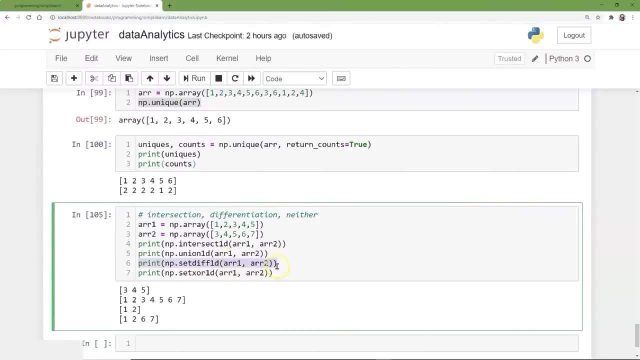 We can see the difference: what's in array 1, but not array 2, so set diff 1D and then set XOR: what is not in 1, but is in 2, and what is not in 2, but in 1.. 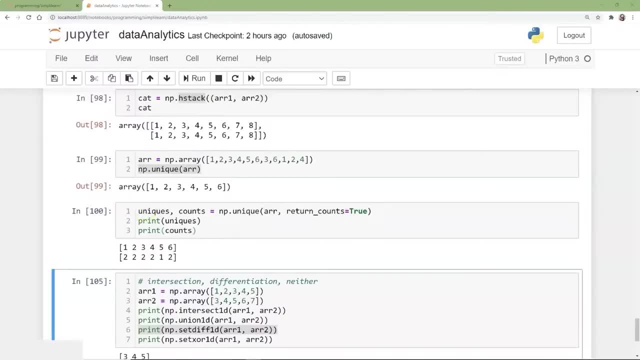 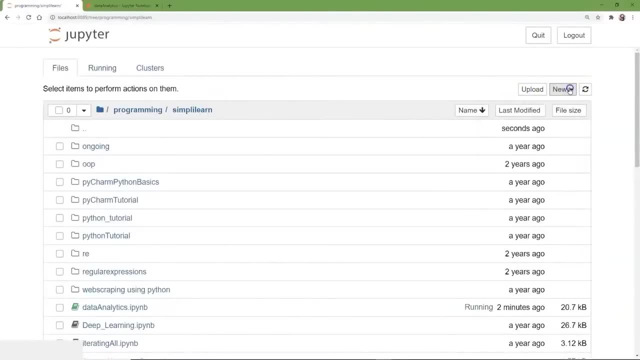 So we dug a lot in NumPy because we were talking. there's a lot of different little mathematical things going on in NumPy. A lot of this can also be done in pandas, although usually the heavy lifting is left for NumPy because that's what it's designed for. 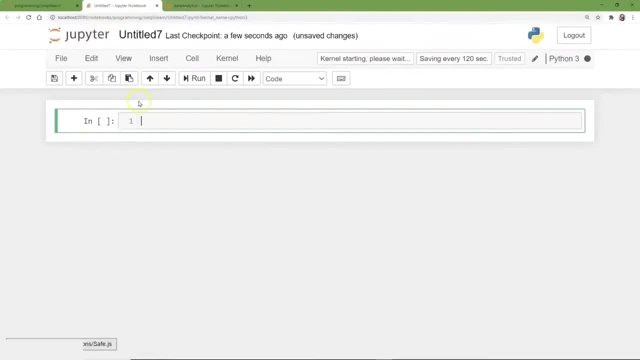 Let's go ahead and open up another Python 3 setup in here. For what happens when you want to display this? This is where it starts getting, in my opinion, a little fun, because you're actually playing with it and you have something to show people. 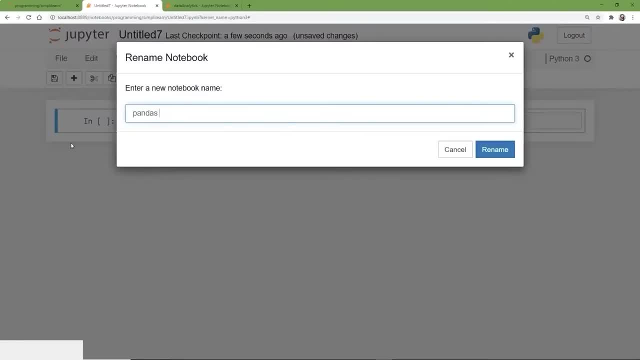 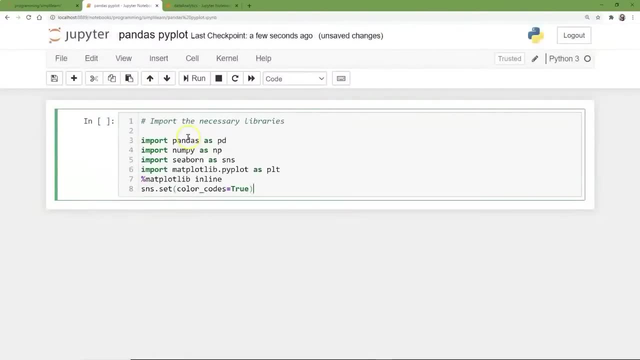 And we'll go ahead and rename this. we're going to call this pandas and pyplot, So pandas, pyplot, just so we can remember for next time. And we want to go ahead and import the necessary libraries. We're going to import pandas as pd. 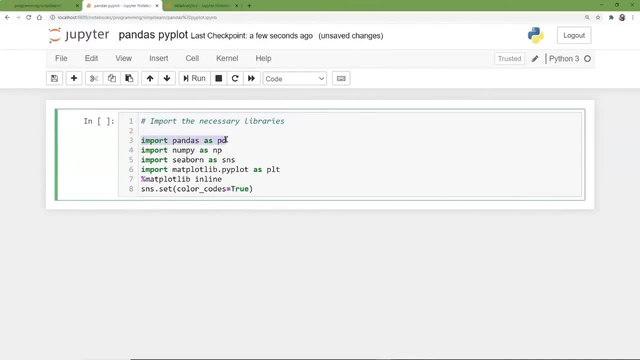 Now, remember, this is a data frame, so we're talking rows and columns and you'll see how pandas work so nicely when you're actually showing data to people. And then we're going to have NumPy in the background. NumPy works with pandas. 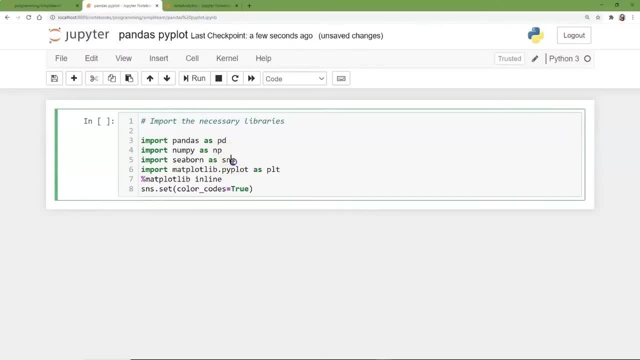 A lot of times you just import them by default. Seaborn sits on top of the Matplot library, So sometimes we use the Seaborn because it kind of extends. it's one of the hundred packages that extends the Matplot library. 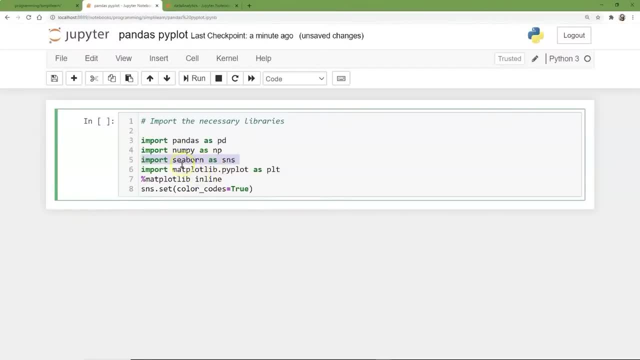 Probably the most commonly used, because it has a lot of built in functionality, Almost by default. I usually just put Seaborn in there in case I need it a bit, But unfortunately I don't always want to do this in a bugchtopx, so I'll do this in success. 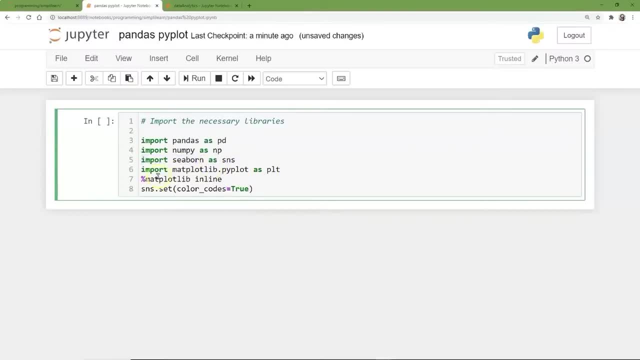 Instead I'll take it by default, I'll take it by exhaust and then some effort and then some distortion and none of the work unless it's through Windows in there in case i need it. and of course we have matplot library as piplot, as plt and note. we have 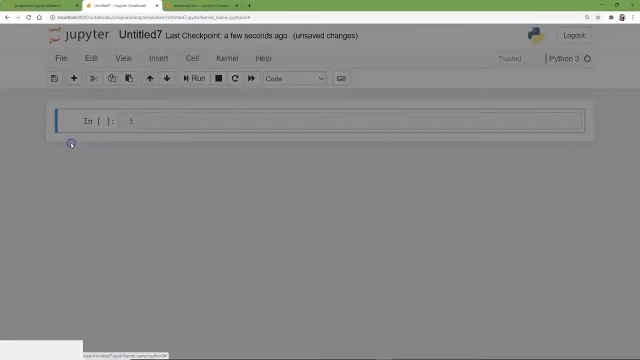 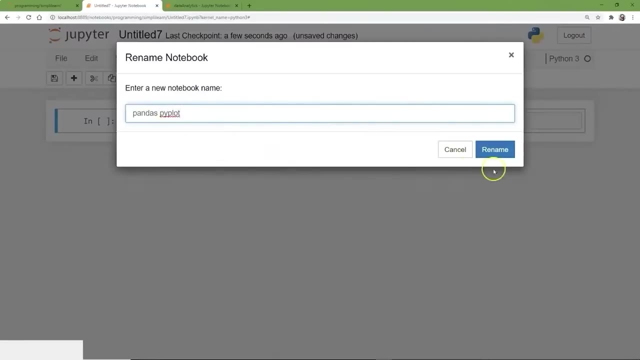 because you're actually playing with it and you have something to show people, And we'll go ahead and rename this. We're going to call this pandas and pyplot, So pandas, pyplot, just so we can remember for next time. And we want to go ahead and import. 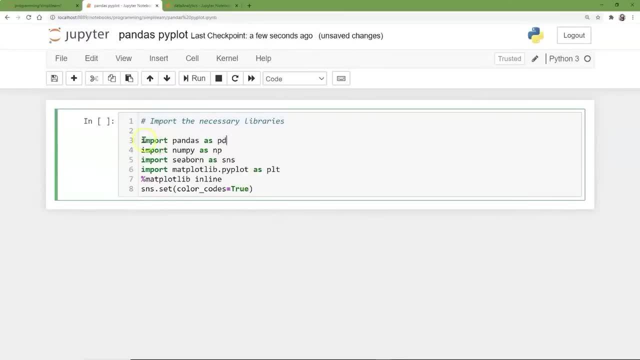 the necessary libraries. We're going to import pandas as PD. Now, remember, this is a data frame, So we're talking rows and columns and you'll see how pandas work so nicely when you're actually showing data to people. And then we're going to have NumPy in the background. 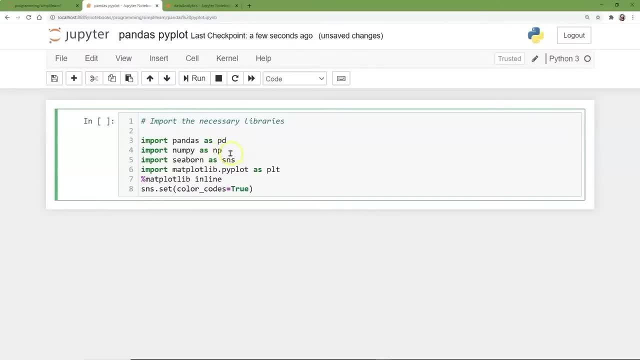 NumPy works with pandas, So a lot of times you just import them by default. Seaborn sits on top of the Matplot library, So sometimes we use the Seaborn because it kind of extends. It's one of the hundred packages. 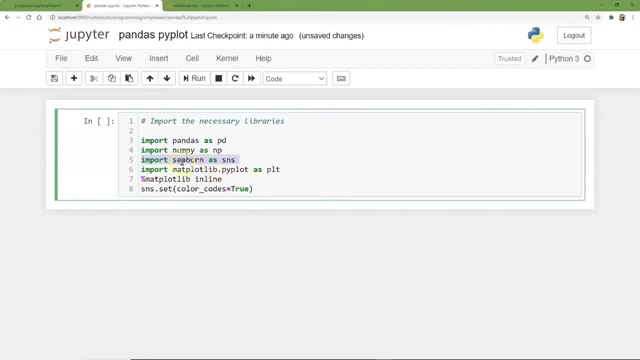 that extends the Matplot library, Probably the most common used because it has a lot of built-in functionality, Almost by default. I usually just put Seaborn in there in case I need it And of course we have Matplot library as pyplot, as PLT. 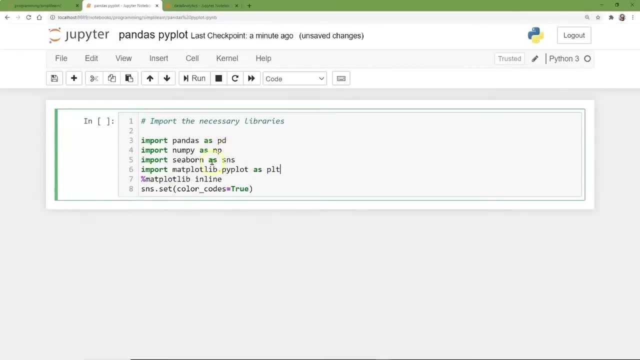 And note we have as PD, as NP, as SNS, as PLT. Those are pretty standard. If you're doing your imports, I would probably keep those, just so other people can read your code and it makes sense to them. That's pretty much a standard nowadays. 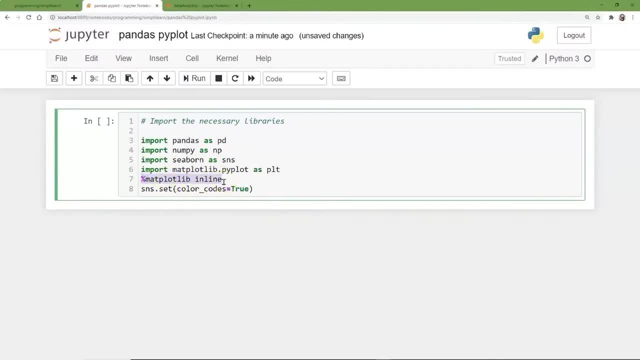 And then we have this strange line here. It says Ambersine Matplot library inline. That is for Jupyter Notebook only. So if you're running this in a different package you'll have a pop-up when it goes to display the Matplot library. 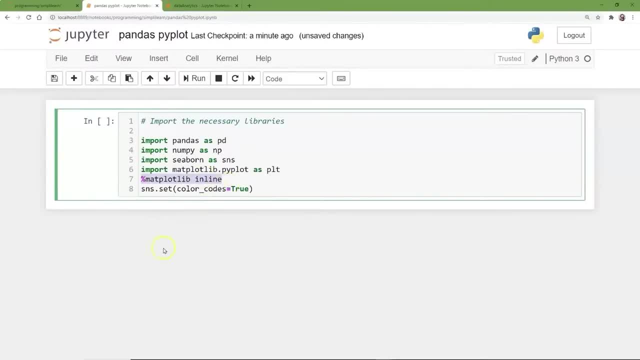 You can, with the most current version of Jupyter, usually leave that out and it will still display it right on the page as we go. That's what that looks like, And then we're going to go ahead and just do the Seaborn, the snsset. 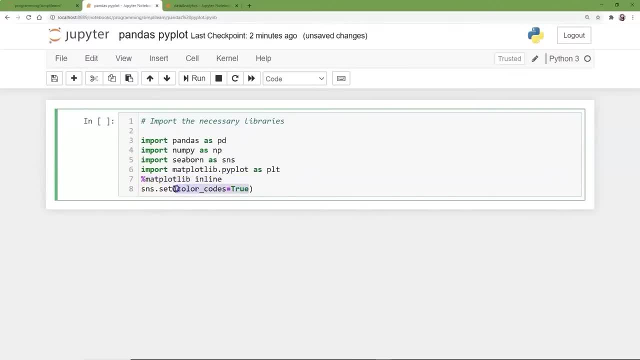 and we're going to set the color codes equals true, Let them just keep the default ones, so we don't have to think about it too much. And we, of course, have to run this. The reason we run this is because these values are all set. 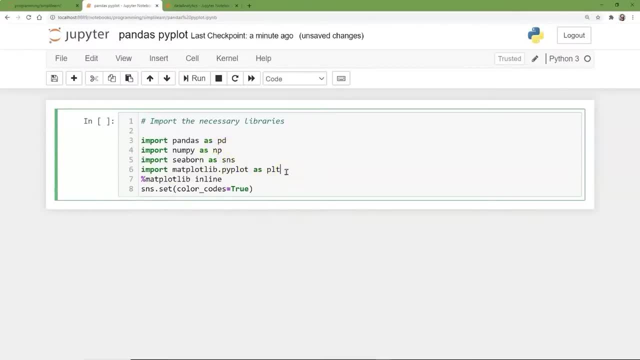 as pd, as np, as sns, as plt. those are pretty standard. so when you're doing your imports, i would probably keep those, just so other people can read your code and it makes sense to them. that's pretty much a standard nowadays. and then we have the strange line here. uh, it says: 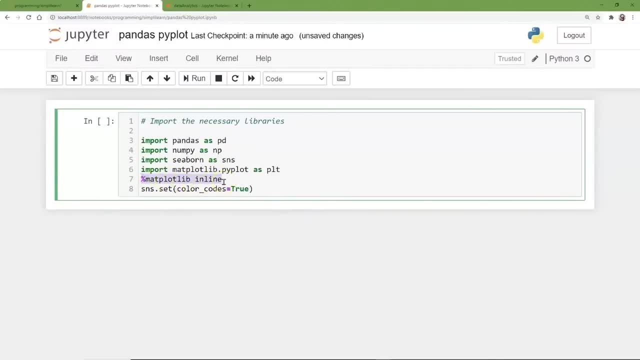 ambersign matplot library inline. that is for jupyter notebook only. so if you're running this in a different package you'll have a pop-up when it goes to display the matplot library. you can, with the most current version of jupyter, usually leave that out and it will still display. 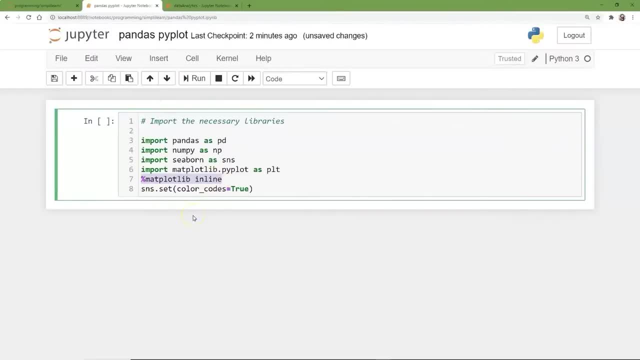 it right on the page as we go and we'll see what that looks like. and then we're going to go ahead and just do the seaborn, the snsset, and we're going to set the color codes equals true. let them just go ahead and do that. and then we're going to go ahead and just do the color codes equals true. 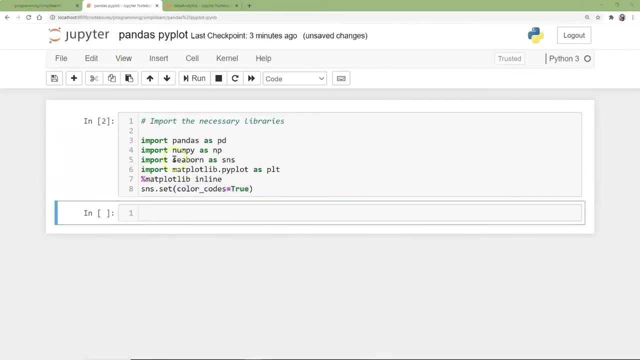 and we're going to go ahead and just do the color codes equals true, and we're going to set the color. just keep the default one. so we don't have to think about it too much. and we of course, have to run this. the reason we run this is because these values are all set. 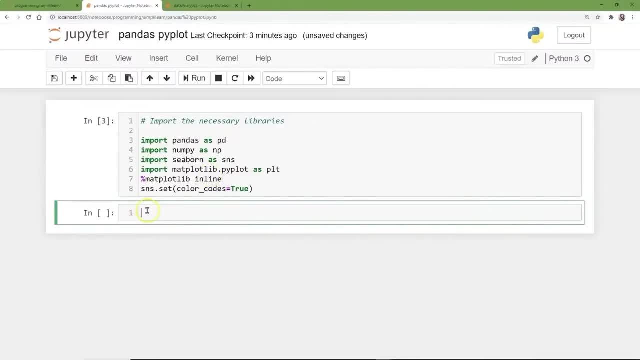 if we don't run this and i access one of these afterward, it'll crash. the cool thing about jupyter notebooks is if you forgot to import one of these, you forgot to install it, because you do have to install this under your anaconda setup or whatever setup you're in. you can flip over to anaconda and 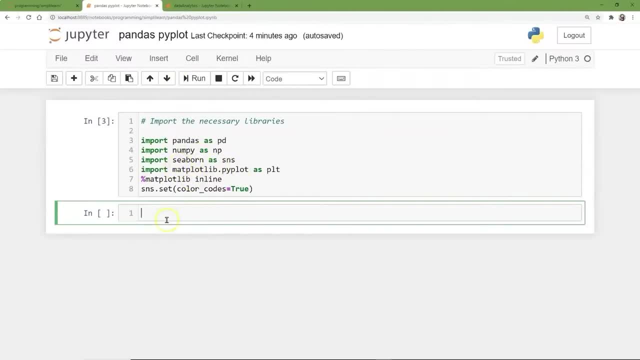 run your install for these and then just come back and run it and you're good to go. you don't have to close anything out and we'll go ahead and paste this one in here real quick: where we have car equals, pd, dot, read underscore csv, and then we have the actual path, this path. 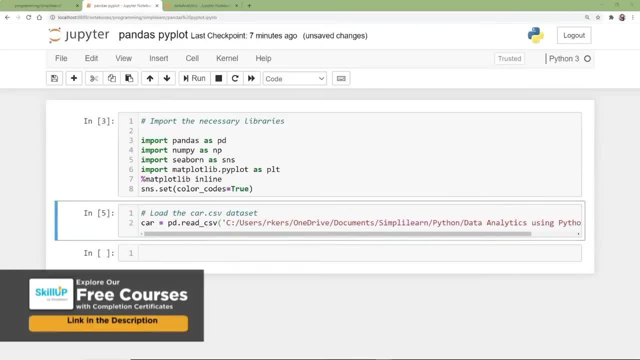 of course, will vary depending on what you are working with, so it's wherever you save the file at, and you can see here i have, like my one, drive documents. simply learn python data analytic using python. slash. car equals pd dot. read underscore csv and then we have the actual path, this path of 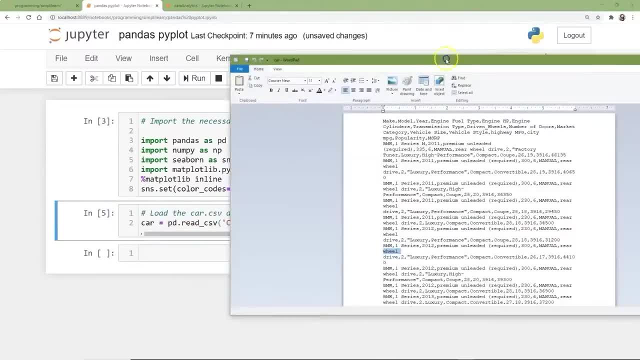 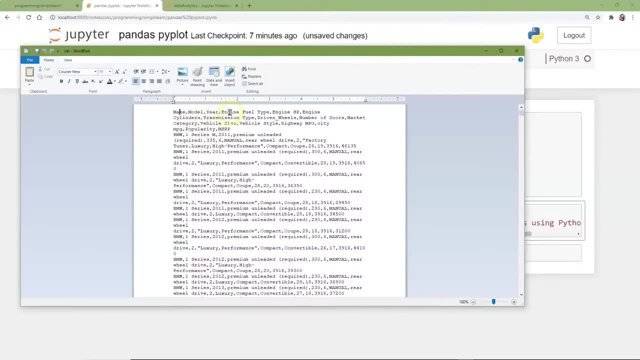 course is pd dot. read underscore csv. it's quite a long file. when we open that up, what we get is we get a csv file and we have the make, the model, the year, the engine fuel type, engine horsepower, cylinders and so on, and this is just a comma separated file, so each row is like a row of data. 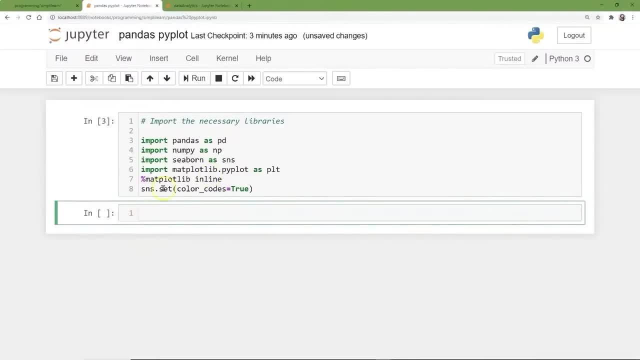 If we don't run this and I access one of these afterward, it will crash. The cool thing about Jupyter Notebooks is if you forgot to import one of these, if you forgot to install it, because you do have to install this under your Anaconda setup. 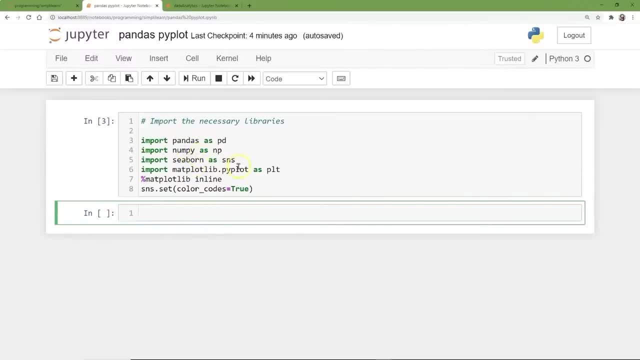 or whatever setup you're in. you can flip over to Anaconda and run your install for these And then just come back and run it. You don't have to close anything out, And we'll go ahead and paste this one in here real quick, where we have. 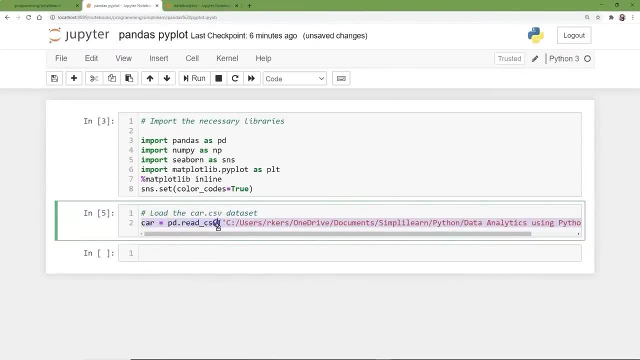 car equals pd dot. read underscore csv, and then we have the actual path. This path, of course, will vary depending on what you are working with, So it's wherever you saved the file at And you can see here I have my OneDrive documents- Simply Learn. 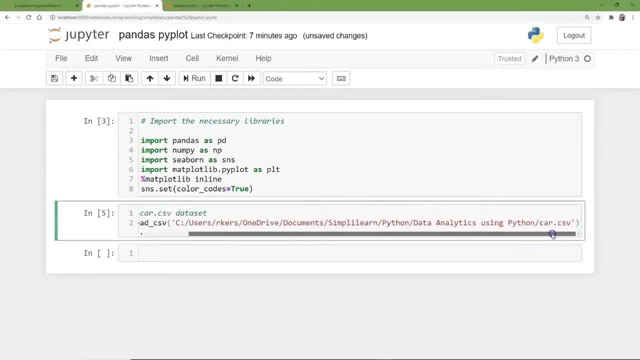 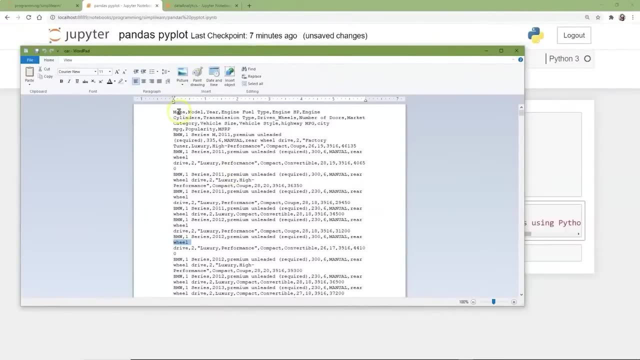 Python Data Analytic using Python slash car csv. It's quite a long file. When we open that up, what we get is we get a csv file and we have the make, the model, the year, the engine fuel type. 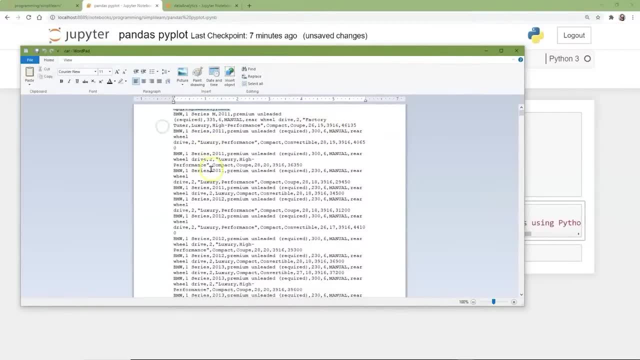 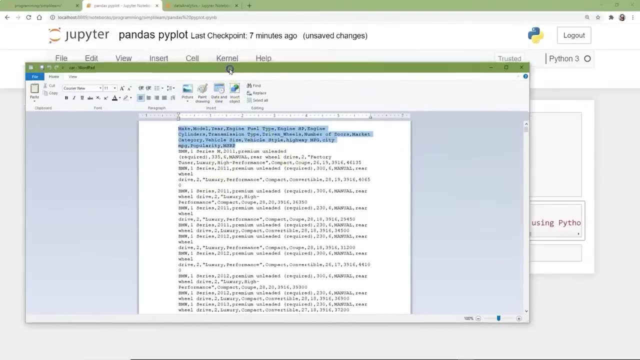 engine, horsepower, cylinders and so on, And this is just a comma separated file, So each row is like a row of data. think of it as a spreadsheet- and then each one is a column of data on here And, as you can see right here, it has the 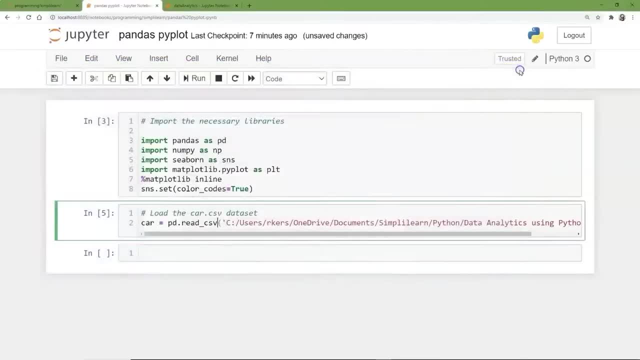 make model, so it has columns for a header on here. Now your pandas just does an excellent job of automatically pulling a lot of this in. So when you start seeing the pandas on here, you realize that you are already like halfway done with getting your data in. 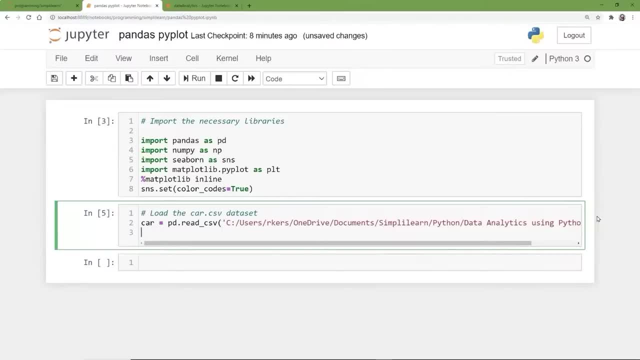 I just love pandas. for that reason, NumPy also has it. You can load a csv directly into NumPy. but we're working with pandas and this is where it really gets. cool is I can come down here and I can print: remember our print statement. we can actually get rid of it. 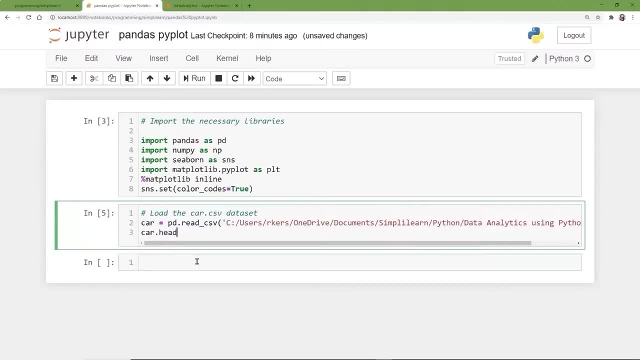 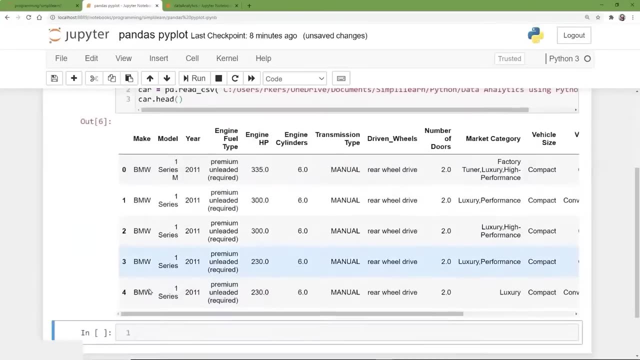 and we're just going to do car head because it's going to print that out. The head is going to print the top values of that data file we just ran in And so you can see right here it does a nice print out, It's all nice and in line. 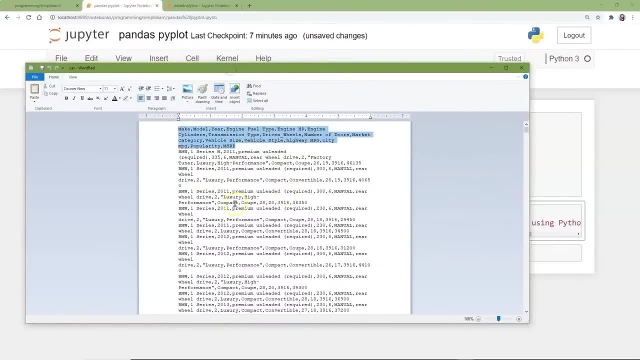 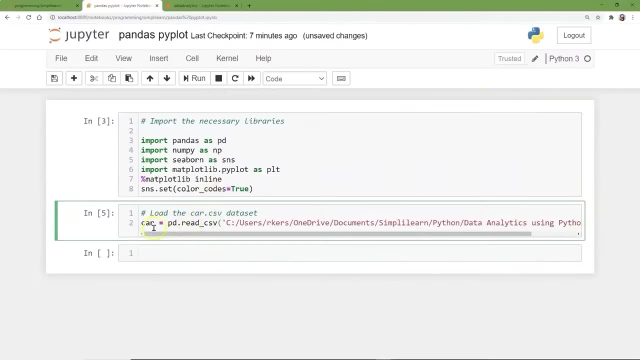 think of it as a spreadsheet, and then each one is a column of data on here and, as you can see right here, it has the make model, so it has columns for a header on here. Now, your pandas just does an excellent job of automatically pulling a. 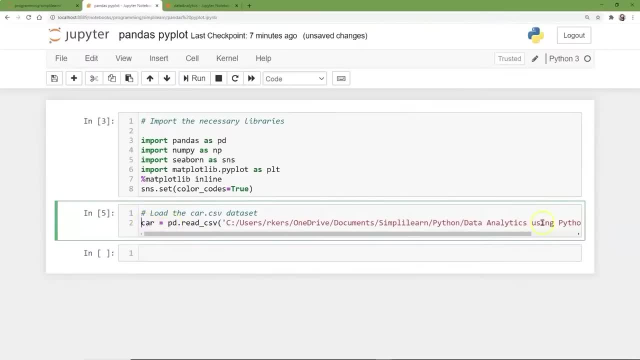 lot of this in. So when you start seeing the pandas on here, you realize that you are already like halfway done with getting your data in. I just love pandas for that reason. NumPy also has it. You can load a CSV directly into NumPy. but we're working with pandas and this is where it really. 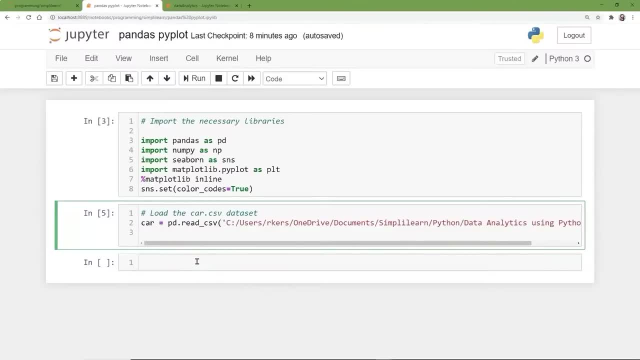 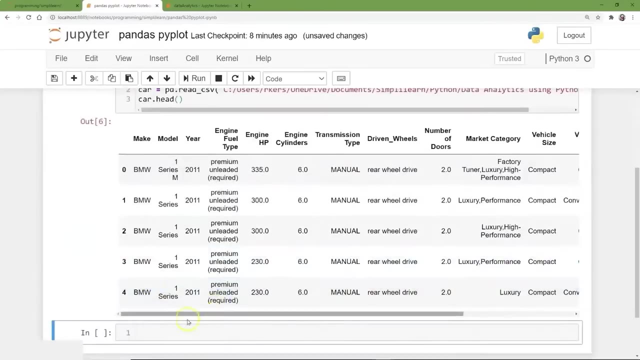 gets cool is I can come down here and I can print. You remember our print statement. We can actually get rid of it and we're just going to do car head because it's going to print that out. The head is going to print the top values of that data file we just ran in and so you can see right here it does. 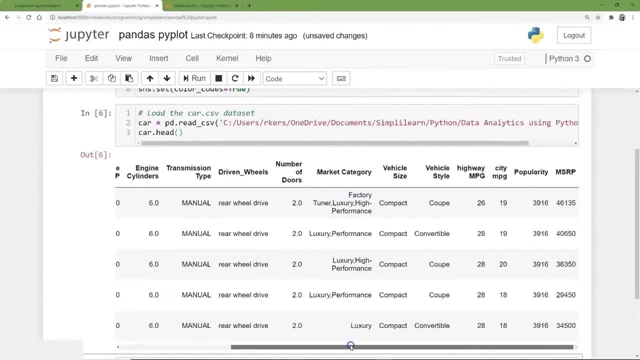 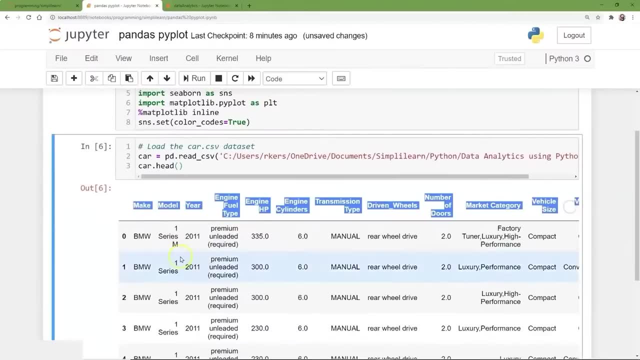 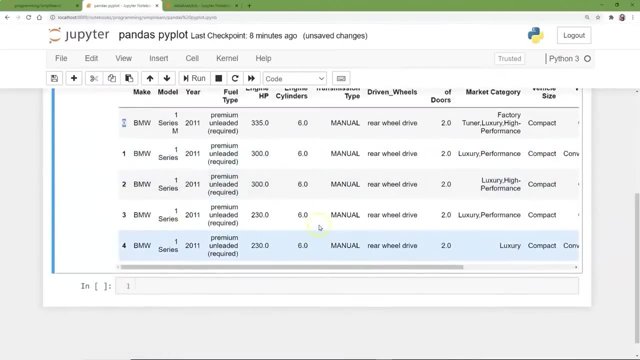 a nice printout. It's all nice and in line because we're in Jupyter Notebook. I can scroll back and forth and look at the different data and, just like we expected, we have our column and it brought the header right in. One thing to note is the index. it automatically created an index- 0, 1, 2, 3, 4 and so on- and we're just 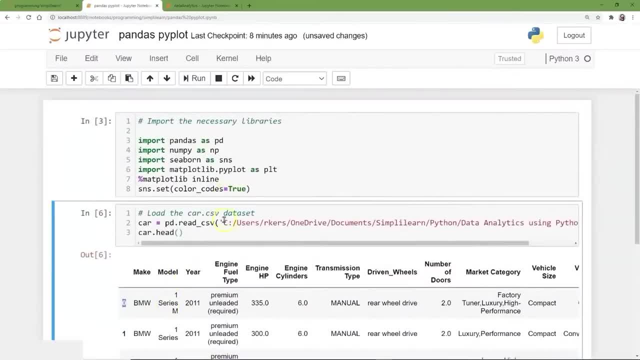 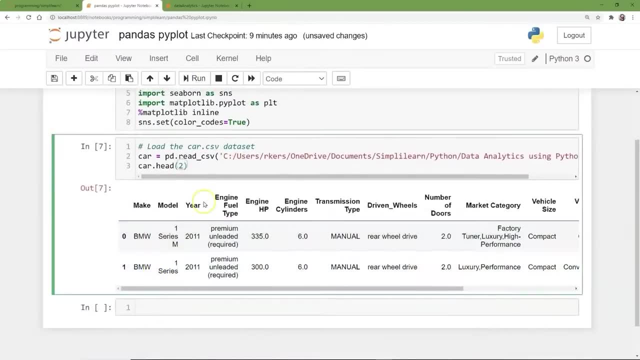 looking at the head. so we got 0, 1, 2, 3, 4.. You can change this. You might want to just look at the top two. We can run that. There's our top two BMWs. Another thing we can do is, instead of head, we can. 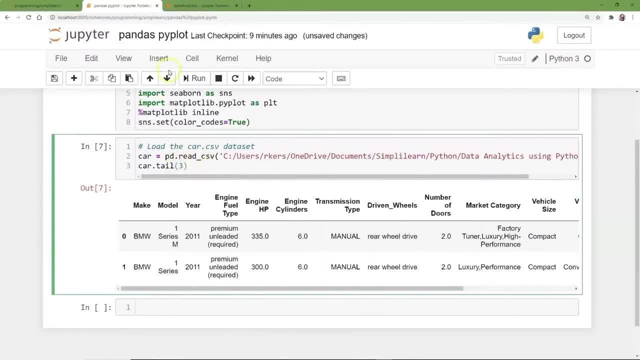 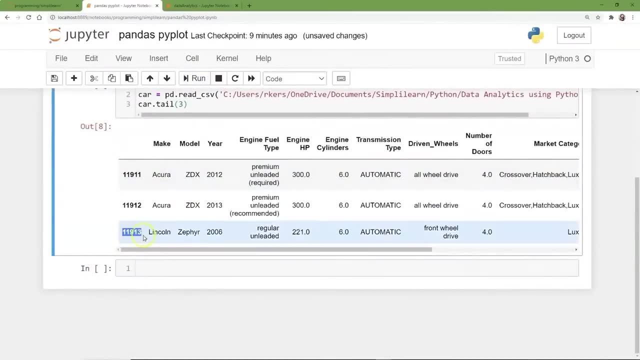 do tail and look at the last three values that are in that data file and you can see right here. it numbered them all the way up to eleven thousand nine hundred and thirteen. Oh my goodness, they put a lot of data in this file. I didn't even look to see how big the file was, So. 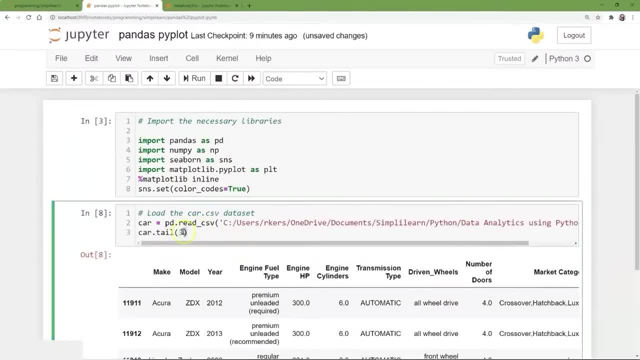 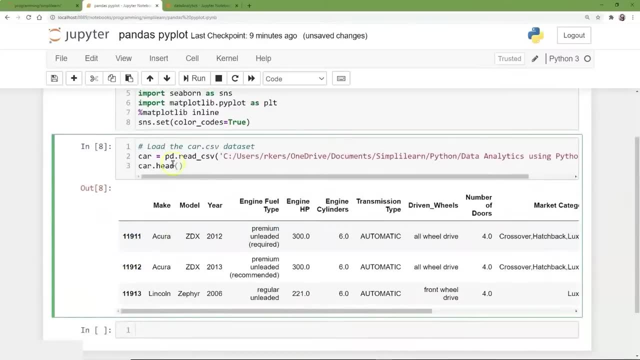 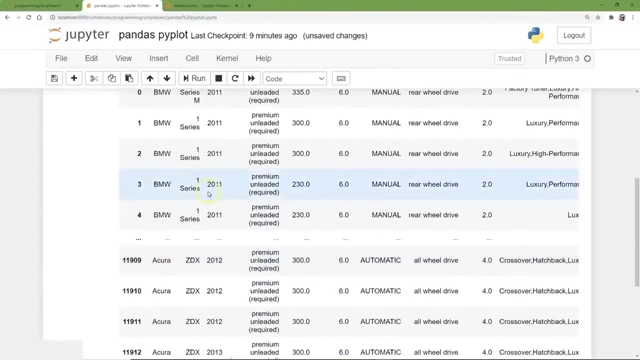 you can really easily get through and view the different data in here. When you're talking about big data, you almost never just print out car. In fact, let's see what happens when we do. If we run this and we just run the car, it's huge. In fact, it's so big that the pandas automatically truncates. 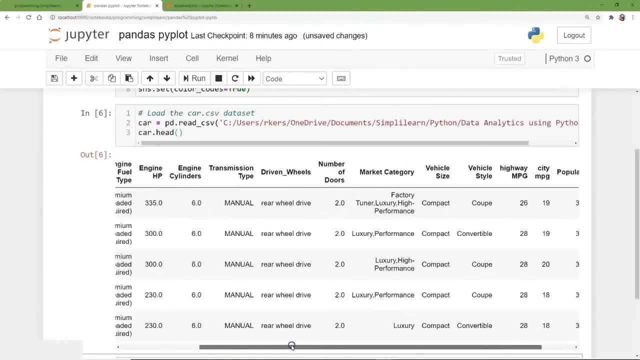 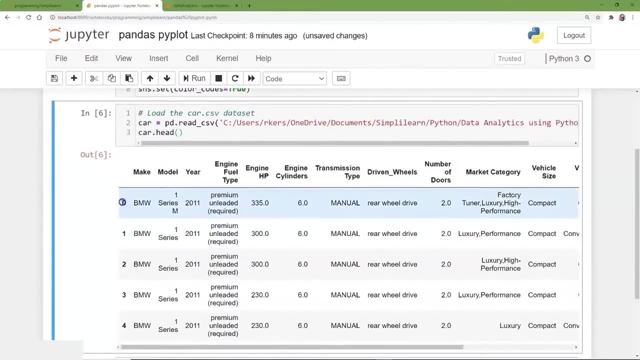 because we're in Jupyter Notebook. I can scroll back and forth and look at the different data and, just like we expected, we have our column and it brought the header right in. One thing to note is the index. it automatically created an index: 0,, 1,, 2,, 3,, 4 and so on. 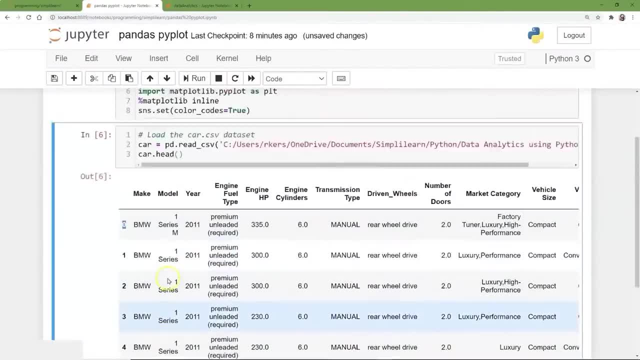 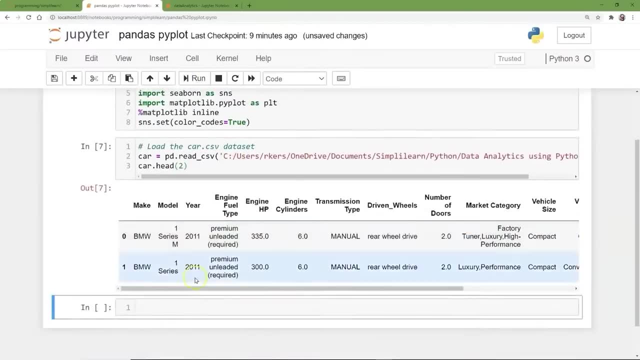 And we're just looking at the head. so we've got 0,, 1,, 2,, 3,, 4.. You can change this. you might want to just look at the top 2. we can run that. there's our top 2 BMWs. 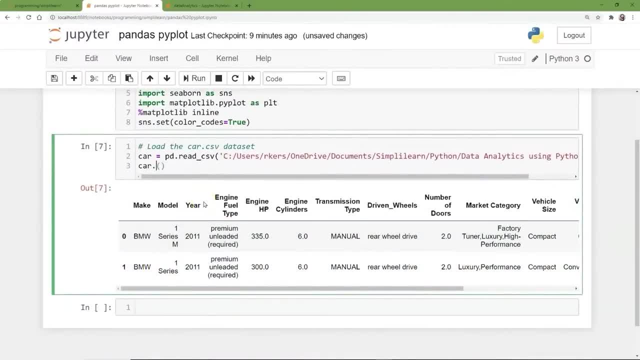 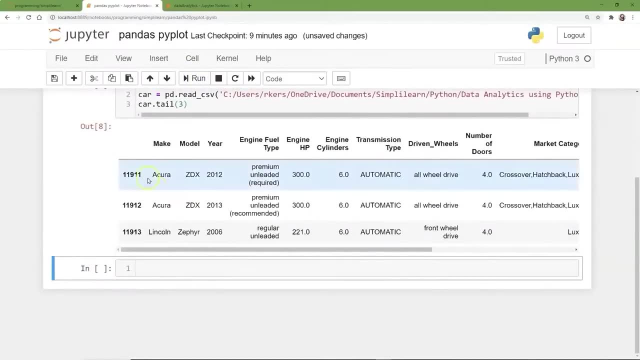 another thing we can do is, instead of head, we can do tail and look at the last 3 values that are in that data file and you can see right here it numbered them all the way up to 11,913.. Oh my goodness, they put a lot of data in this file. 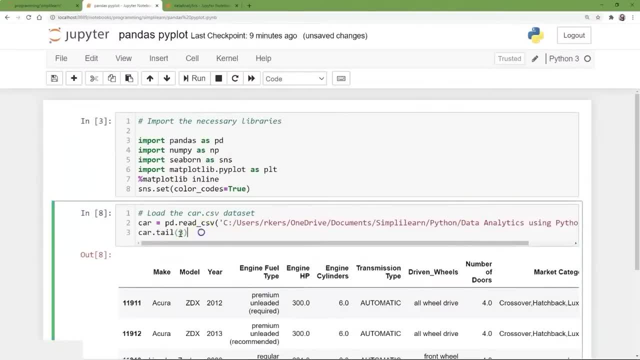 I didn't even look to see how big the file was, So you can really easily get through and view the different data in here. When you're talking about big data, you almost never just print out car. In fact, let's see what happens when we do, If we run this: 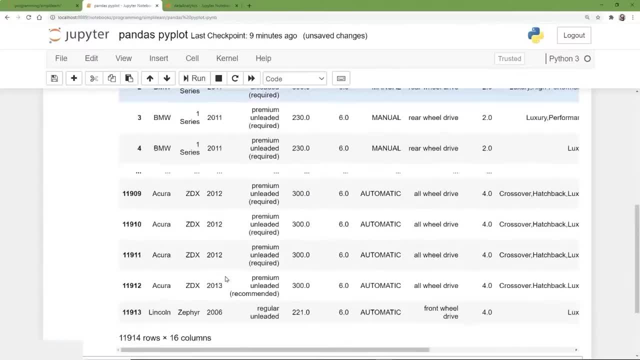 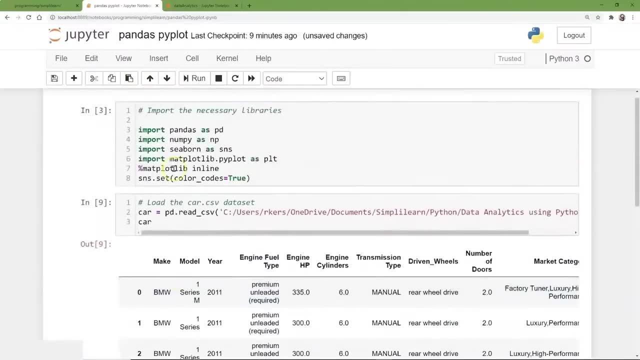 and we just run the car. it's huge. In fact it's so big that the pandas automatically truncates it and just does head plus tail. So you can see the two. So we really don't want to look at the whole thing. I'm going to go back to. let's stick with the head. 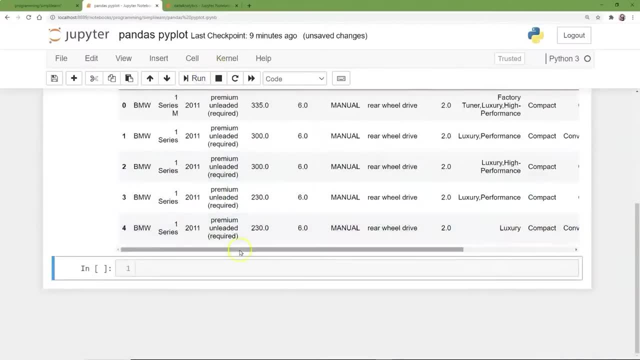 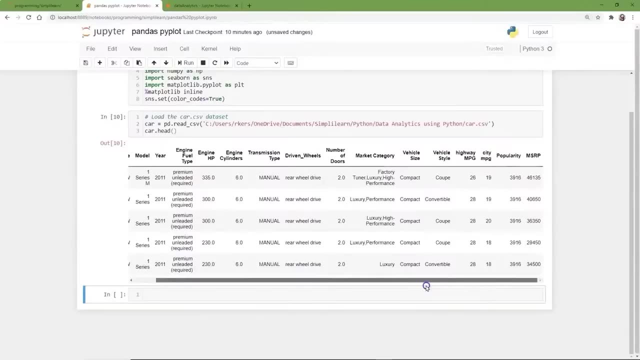 displaying our data. There we go, So there's the head of our data. it gives us a quick look to see what's actually in there. I can zoom out if you want so you can actually get a better view, Although we'll keep it zoomed in so you can see the. 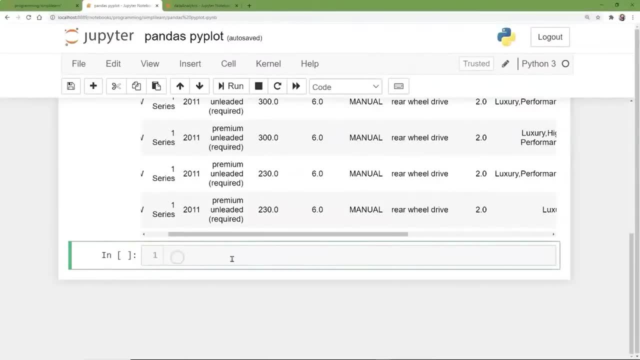 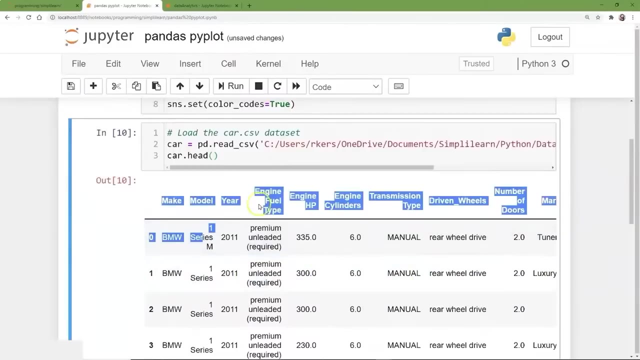 code I'm working on. And then, from the data standpoint, we of course want to look at data types. What's going on with our data? What does it look like? Now, this you show when you're talking to your shareholders. they like to see these nice, easy to read charts. 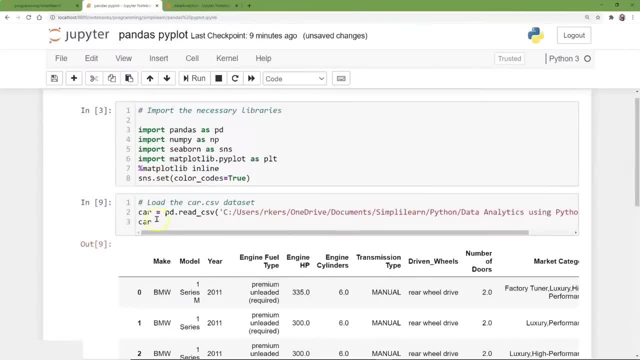 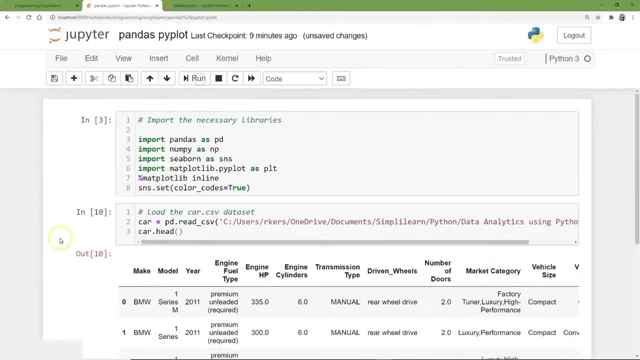 and just does head plus tail so you can see the two. So we really don't want to look at the whole thing. We're going to go back to stick with the head displaying our data. There we go. So there's a head of our data. gives us a quick look to see what's actually in there. I can zoom out if you. 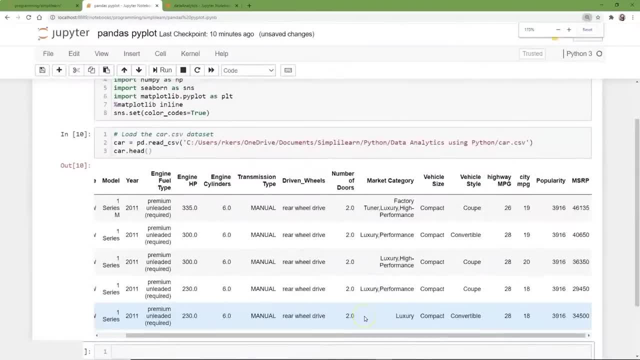 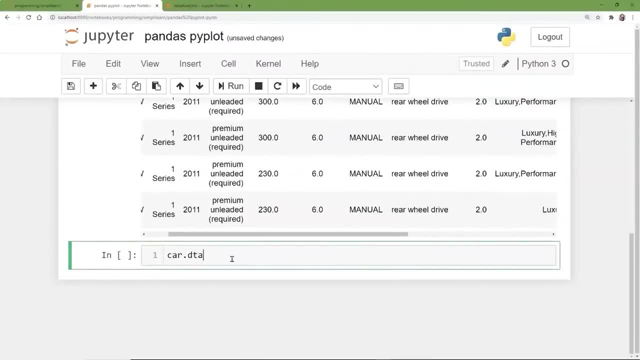 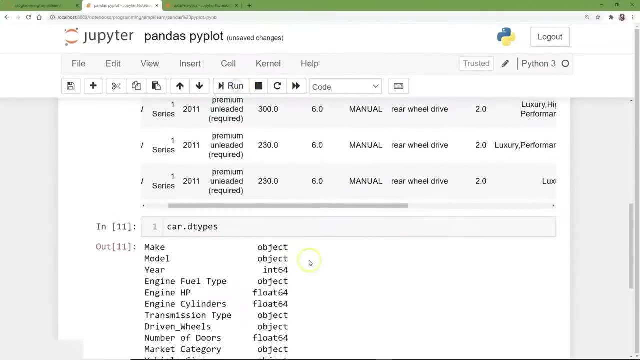 want to actually get a better view, Although we'll keep it zoomed in so you can see the code I'm working on. And then, from the data standpoint, we of course want to look at data types. What's going on with our data? What does it look like? Now? this you know. you show your. 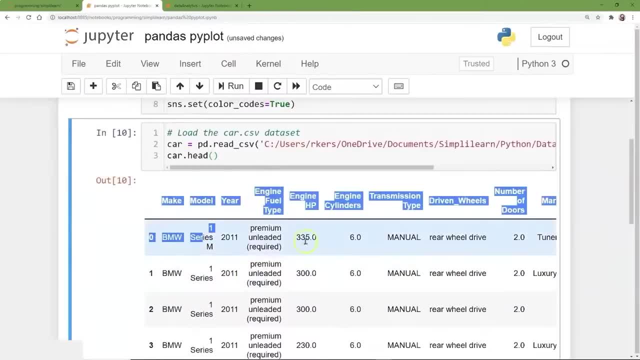 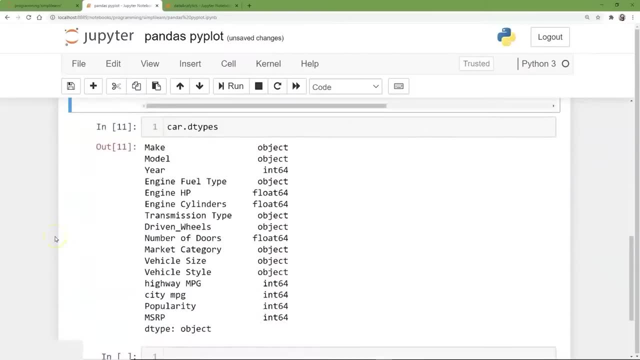 when you're talking to your shareholders. they like to see these nice, easy to read charts. They look like a spreadsheet, So it's a nice way of displaying pieces of the chart. We talk about the data types. Now we're getting into the data science side of it. What are we working with? Well, 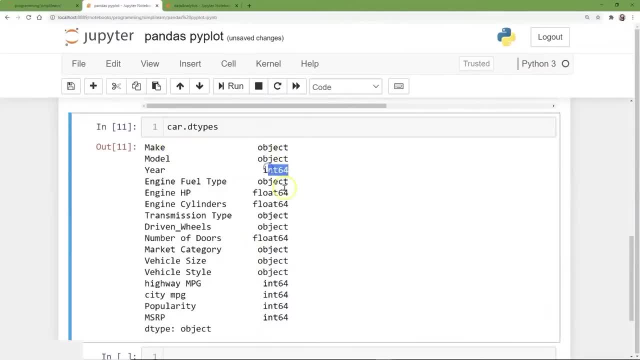 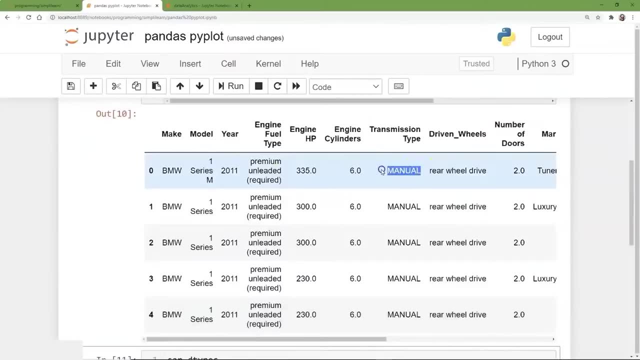 we have make model. We have an integer 64 for the year. Engine field type is an object. If we go up here you can see that they're. most of them are like you know it's a set manual rear wheel drive, So they may be very limited number of types in there And so forth, And you know it's. 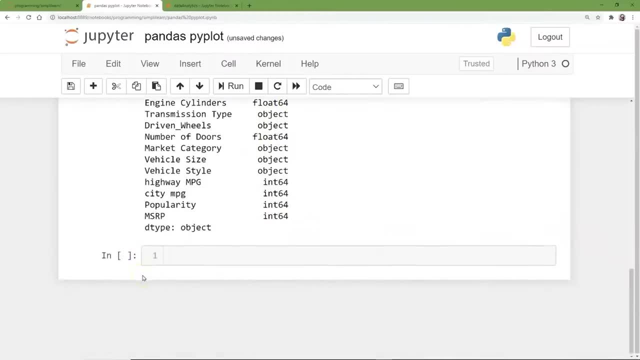 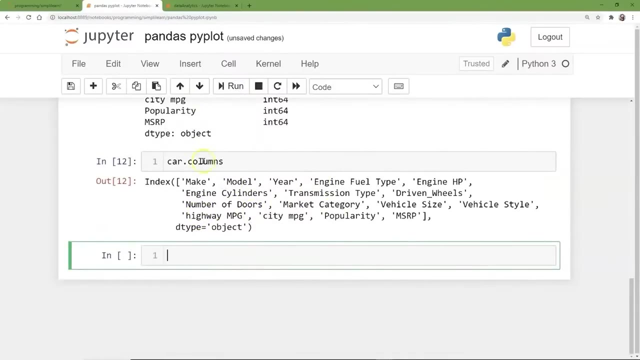 either going to be a float 64, an integer or an object is the way it's going to read it on here. And the next thing you want to know is, like your columns, And since it loaded the columns automatically, we have here the make, the model, the year, the engine, the size, all the way up to the MSRP. And just out of something, 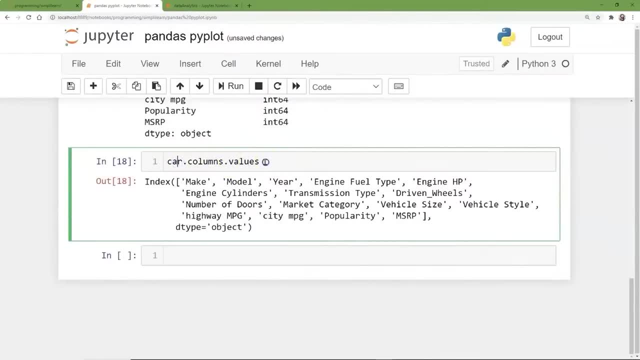 you'll see come up a lot is whenever you're in pandas, you type in dot values, it converts it from a panda's list to a numpy array, And that's true of any of these. So then you end up in a numpy array. So you'll see a little switch in there in the way that the data is actually stored, And 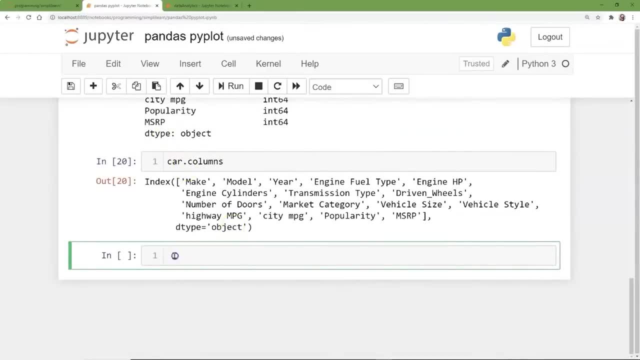 that's true of any of these. In this case, we want carcolumns. You have a total list of your car columns and, like any good data scientist, we want to start looking at analytical summary of the data set. What's going on with our data? So we can start trying to piecemeal it together, So we can do car describe. 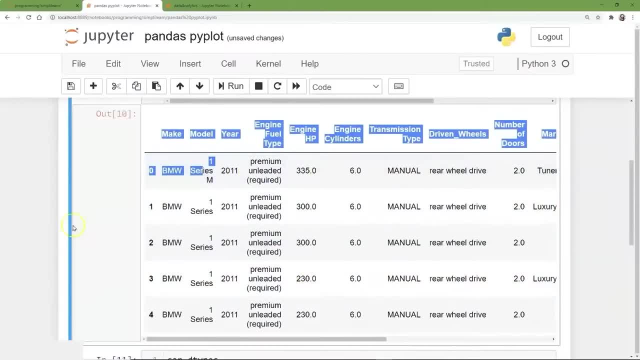 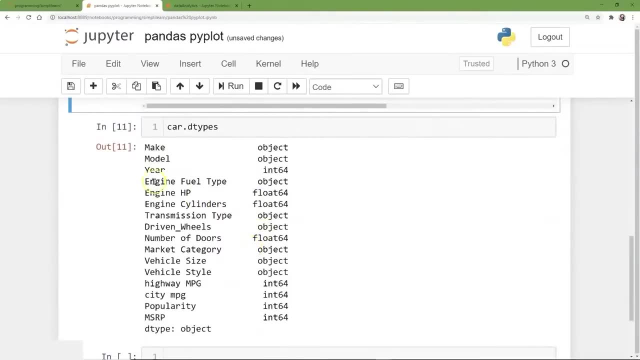 They look like a spreadsheet, So it's a nice way of displaying pieces of the chart. We talk about the data types. now we're getting into the data science side of it. What are we working with? Well, we have make model, we have an integer. 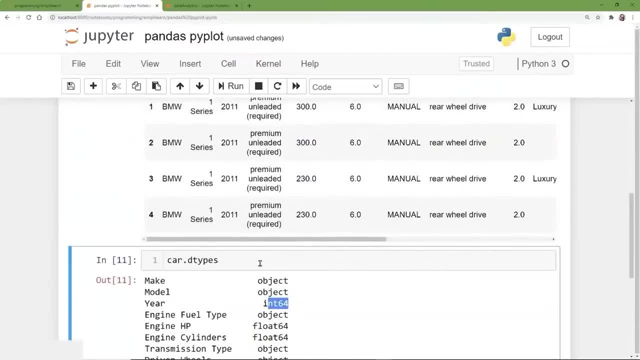 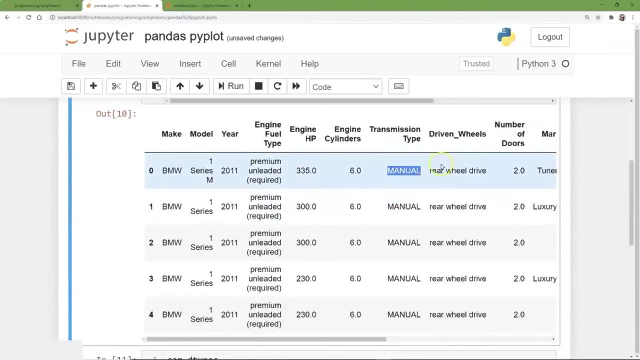 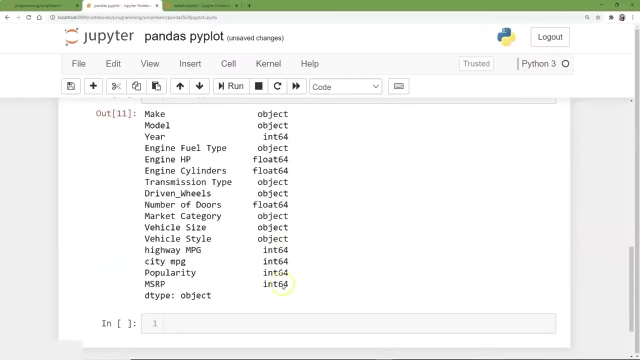 64 for the year Engine fuel type is an object. If we go up here you can see that there most of them are. like you know, it's a set manual rear wheel drive so they might be very limited number of types in there And so forth. 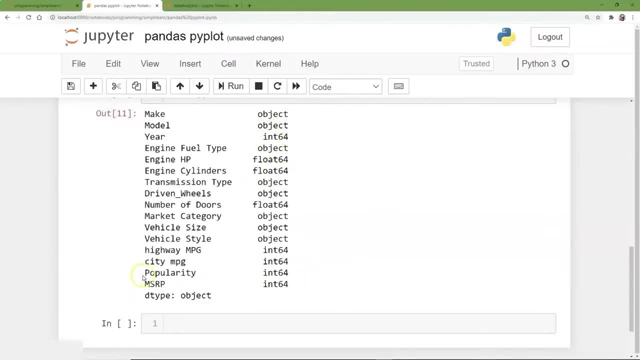 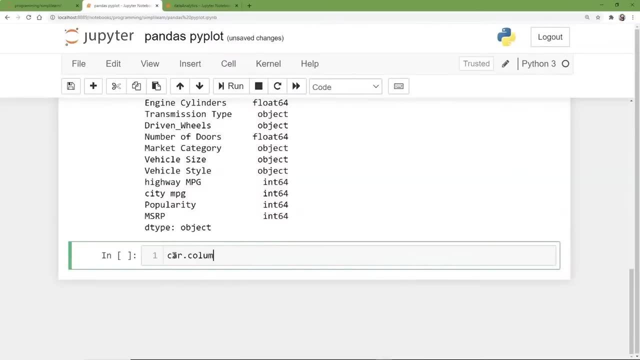 It's either going to be a float 64, an integer or an object is the way it's going to read it on here. And the next thing you're going to want to know is: like your columns and since it loaded the columns automatically, we have here the 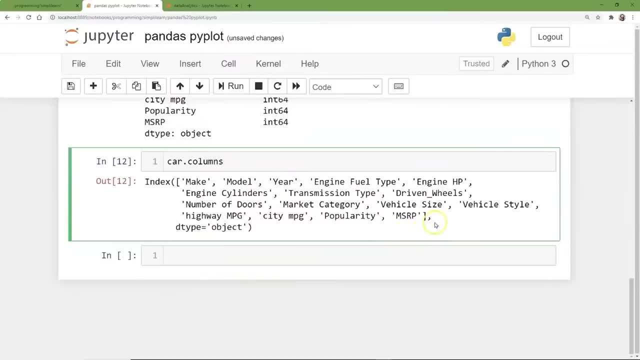 make the model, the year, the engine, the size, all the way up to the MSRP. And just out of something you'll see come up a lot is whenever you're in pandas and you type in dot values, it converts it from a pandas list to a. 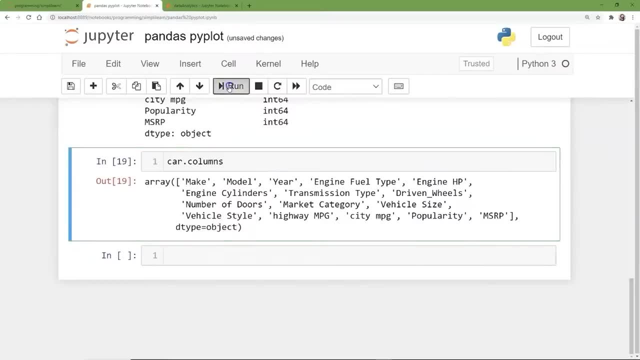 numpy array, And that's true of any of these. You might end up in a numpy array, So you'll see a little switch in there in the way that the data is actually stored, And that's true of any of these. In this case, we want car dot columns. 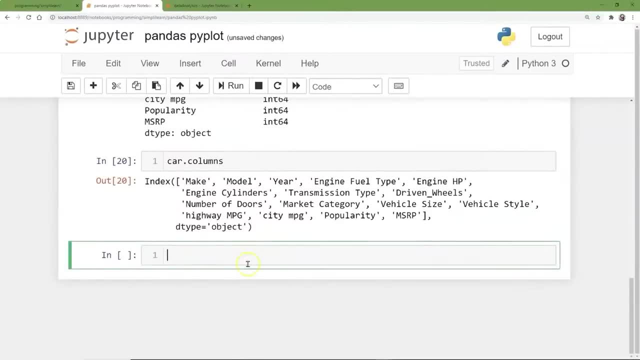 You have a total list of your car columns And, like any good data scientist, we want to start looking at analytical summary of the data set- What's going on with our data- So we can start trying to piecemeal it together, So we can do car. 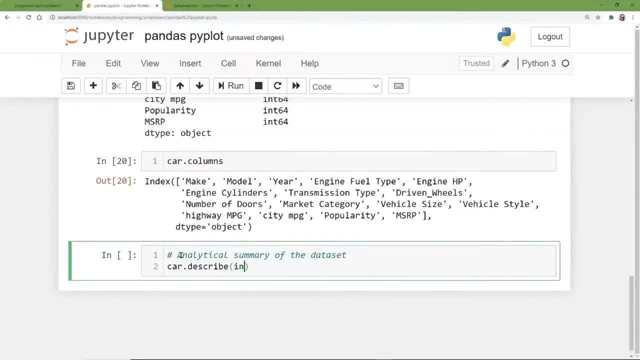 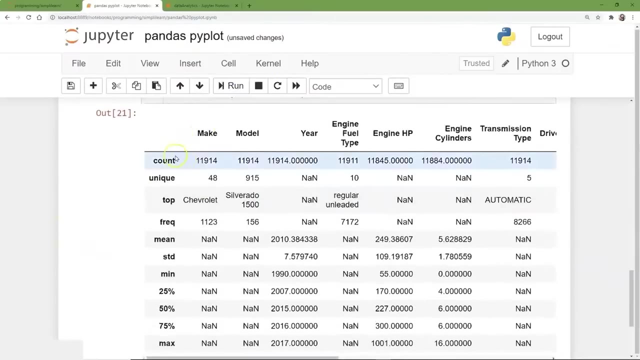 describe and then what we'll do is: we'll do include equals, all. So a nice panda command is to describe your data. If you're working with R, this should start looking familiar And we come down here and you can see count there's. 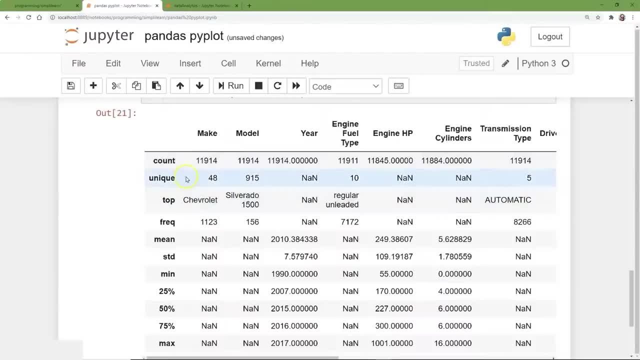 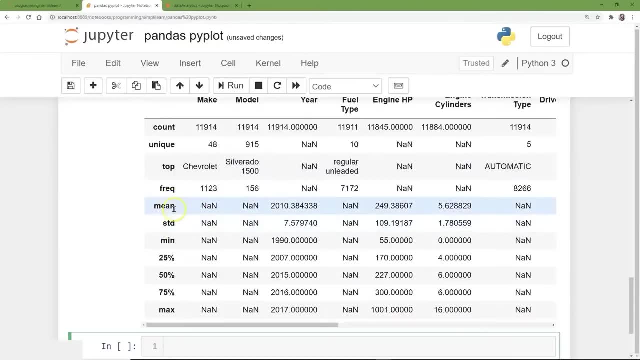 make the model, the year, how many of each one, how many unique values of each one, the top value of each one? what's most common? the frequency, the mean? Clearly, on some of these, it's an object. You really can't tell you what the 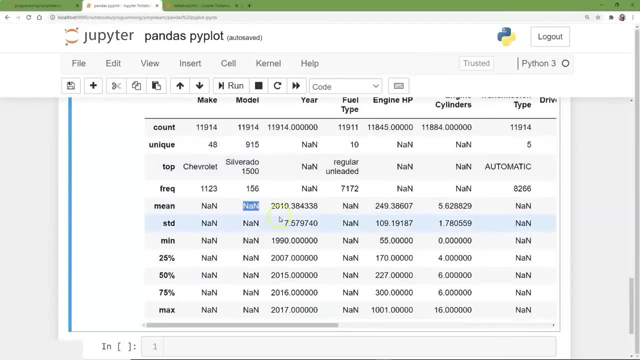 average is. It'd just be the top ones, the average, I guess, The year, what's the average year on there? All this stuff comes down here: Your standard deviation, your minimum value, your maximum value, what's in the lower quarter? 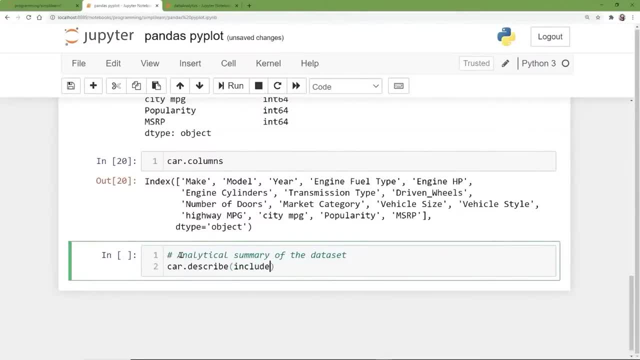 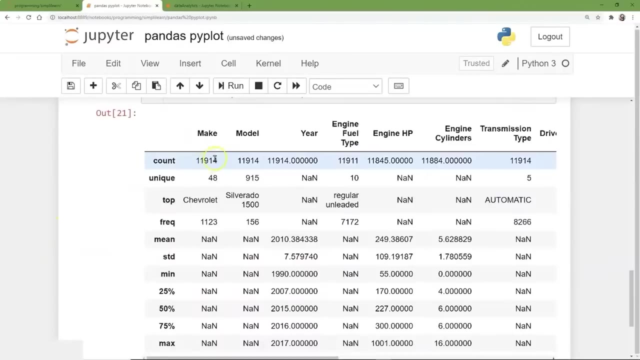 and then what we'll do is: we'll do include equals, all. So a nice panda command is to describe your data. If you're working with R, this should start looking familiar. And we come down here and you can see count there's, make the model, the year, how many of each one, how many unique values of? 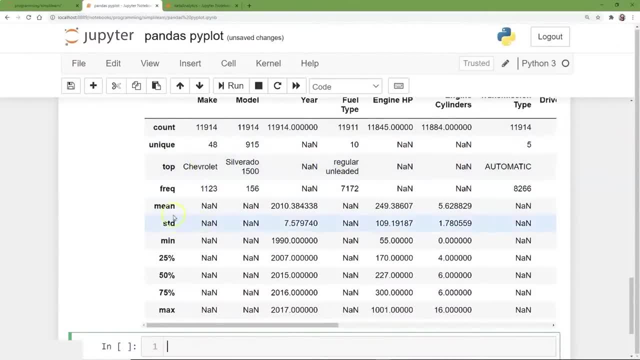 each one. the top value of each one. what's most common: the frequency, the mean. the value of each one. the top value of each one. what's most common: the frequency, the mean. clearly, on some of these it's an object, so it really can't tell you what the average is. It'd. 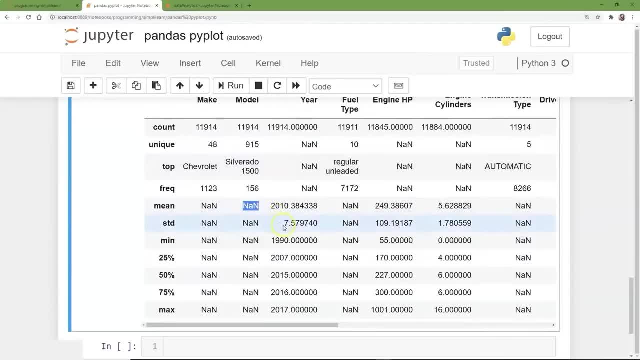 just be the top one's the average, I guess The year, what's the average year on there? All this stuff comes down here: Your standard deviation, your minimum value, your maximum value, what's in the lower quarter 50% mark, where's that line at? and what's in the upper 75%, the top 25% going? 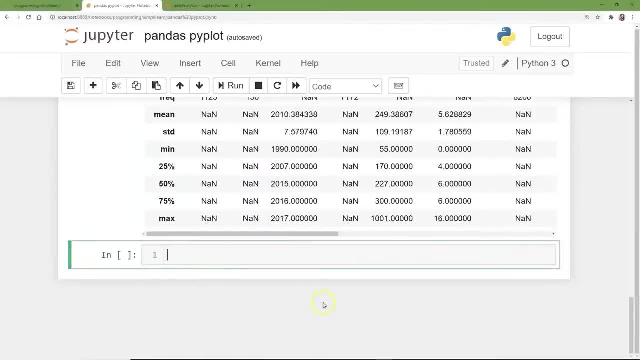 into the max. Now there's a couple of things that we want to look at. We want to look at the next part. This next part is just cool. This is what we always wanted computers to be back like in the 90s. instead of 5,000 lines of code to do this, Maybe not 5,000.. All right, I built my own plot. 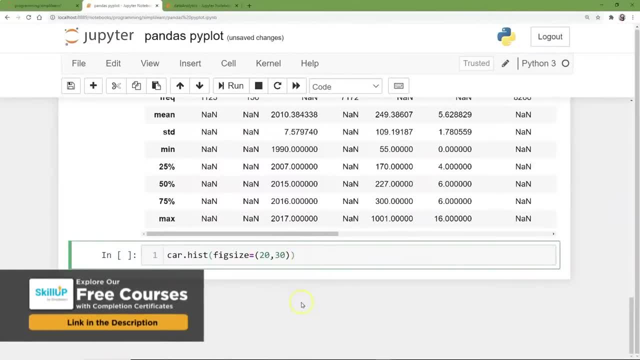 library back in 95 and the amount of code for doing a simple plot was, I don't know, probably about 100 lines of code. This is being done in one line of code. We have our car, which is our pandas. we generated that, it's our data frame and we have dot hist for histograms. 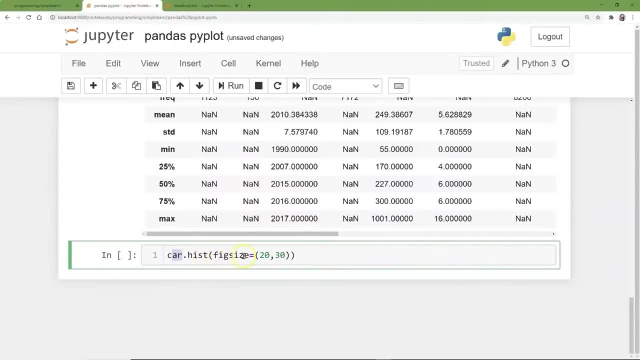 That is the power of Seaborn. Now it's still going to generate a numpy graph, but Seaborn sits on top and then we can do the figure size. This is just so. it fits nicely on the paper on here And we do. 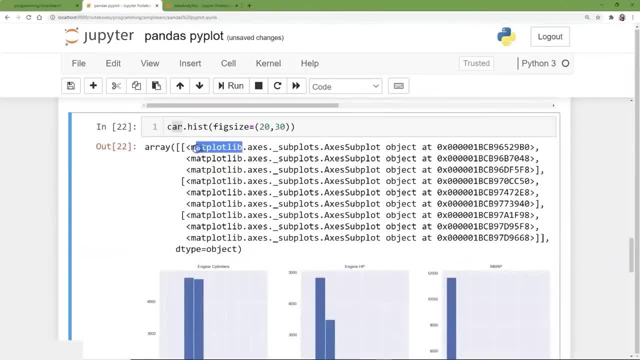 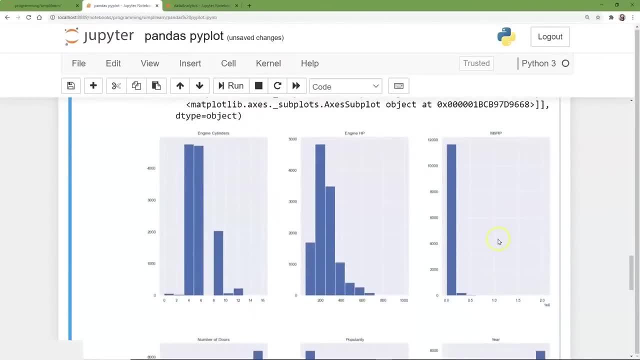 something simple like this and you can see here where it comes up and does a matplot library and does subplots and everything. But we're looking at a histogram of all the different pieces in our database And we have our engine cylinders. that's always a good one because you can see like they have some that are. they had a null on there. 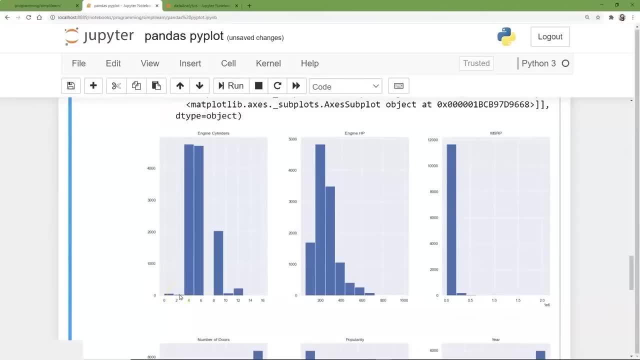 so they came out at zero. Maybe a couple, maybe one of them had a two cylinder engine away back when Four is a common, six a little less common, and then you see the eight cylinder, 12 cylinder engines. well, it's got to be a speedster or something, But you can see, right here, just breaks. 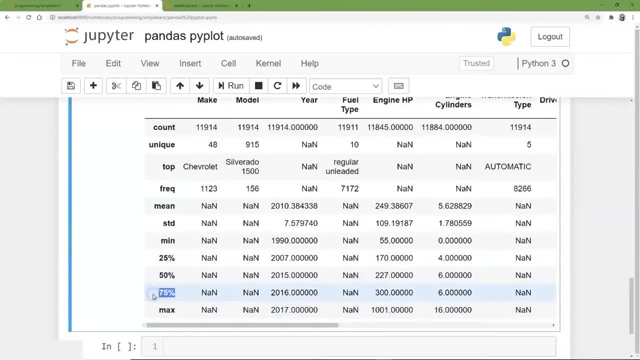 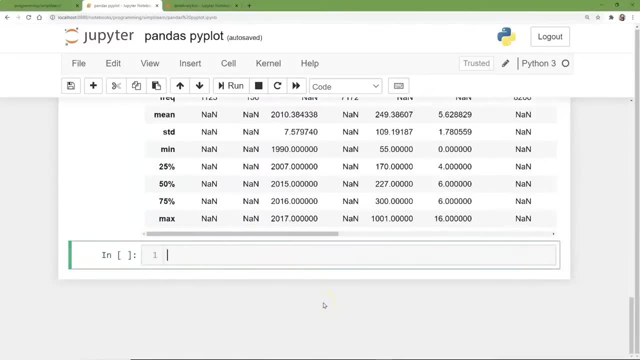 50% mark. where's that line at? and what's in the upper 75%, the top 25% going into the max? Now this next part is just cool. This is what we always do when computers be back like in the 90s. 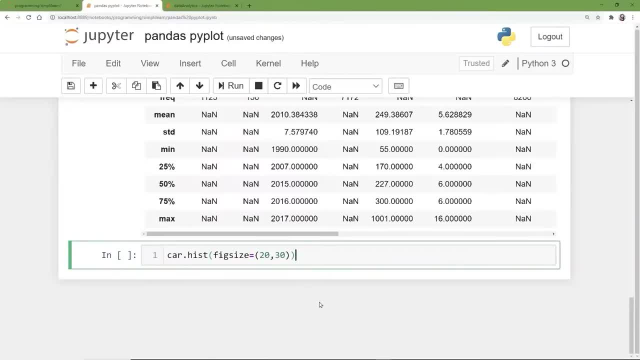 instead of 5,000 lines of code to do this, Maybe not 5,000.. Alright, I built my own plot library back in 95 and the amount of code for doing a simple plot was, I don't know, probably about 100 lines of code. 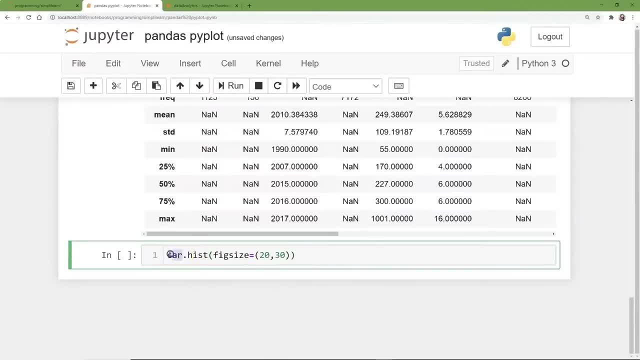 This is being done in one line of code. We have our car, which is our pandas. we generated that, it's our data frame and we have hist for histogram. That is the power of Seaborn. Now it's still going to generate a numpy graph. 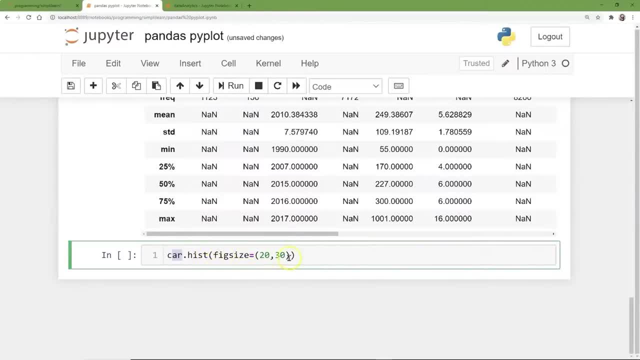 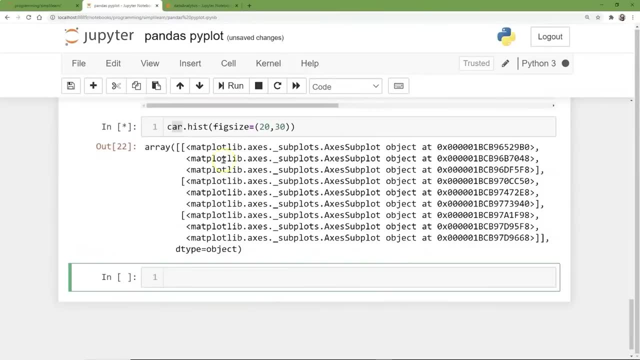 but Seaborn sits on top and then we can do the figure size. This is just so it fits nicely on the paper on here. And we do something simple like this and you can see here where it comes up and it does say matplotlibrary and does subplots. 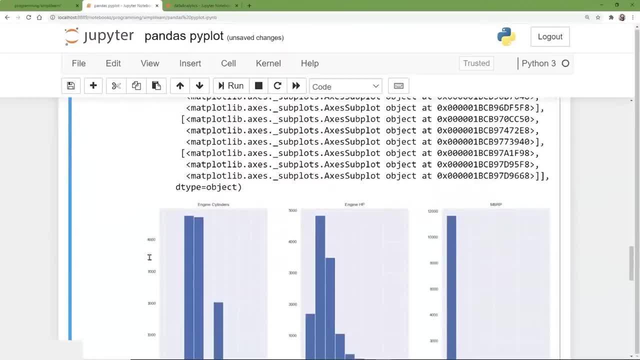 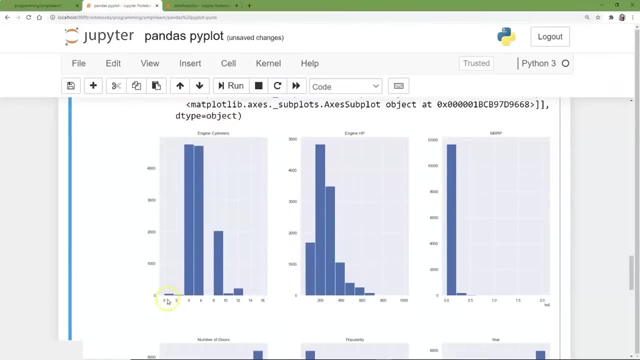 and everything. But we're looking at a histogram of all the different pieces in our database And we have our engine cylinders. that's always a good one, because you can see they have some that had a null on there, so they came out at zero. Maybe a couple, maybe one of them had a two cylinder engine way back when. Four is a common, six a little less common, and then you see the eight cylinder, twelve cylinder engines. boy, that's got to be a speedster or something. 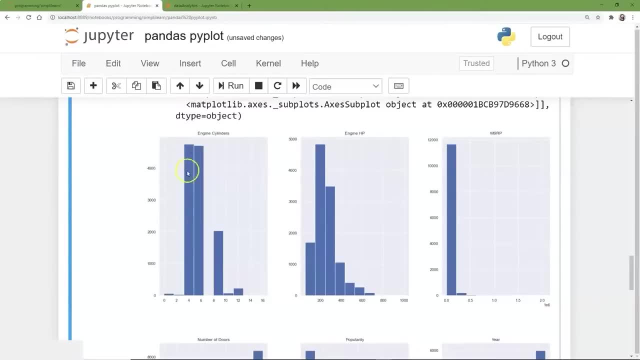 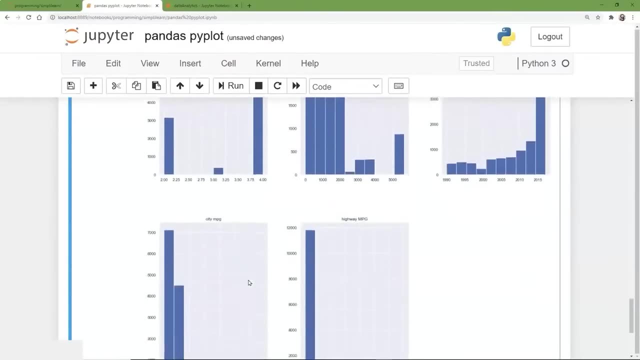 But you can see right here. it just breaks it down. so now you have how many cars with how many, whatever it is- cylinders, horsepower and so on, And it does a nice job displaying it. You can see if you're working with your. 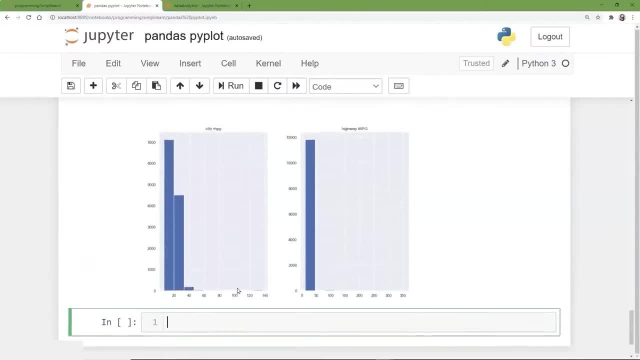 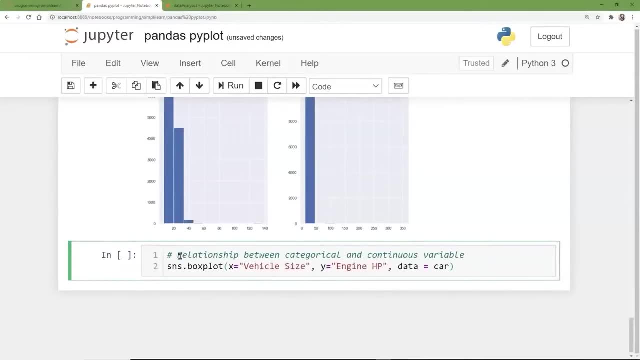 you're going into your demo. it's really nice just to be able to type that in and boom, there it is. They can see it all the way across, And we might want to zero in and use like a boxplot, And this time we'll go ahead and call the. 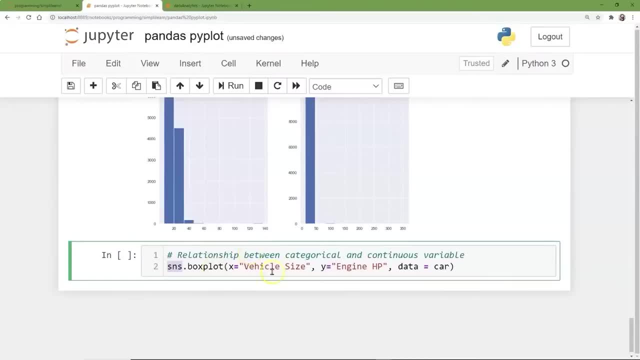 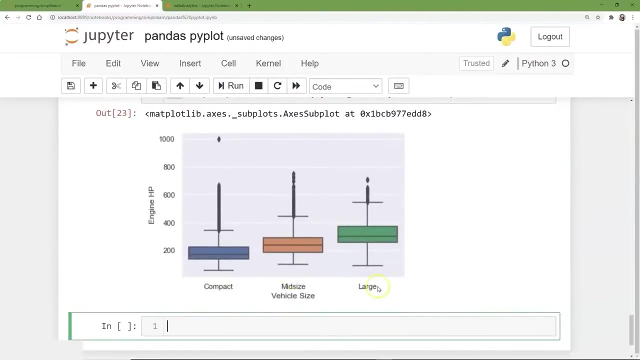 Seaborn SNS boxplot and we're going to go ahead and do vehicle size versus engine horsepower xyplot And the data comes from the car. So if we run this we end up with a nice boxplot. You see our midsize, compact and large. 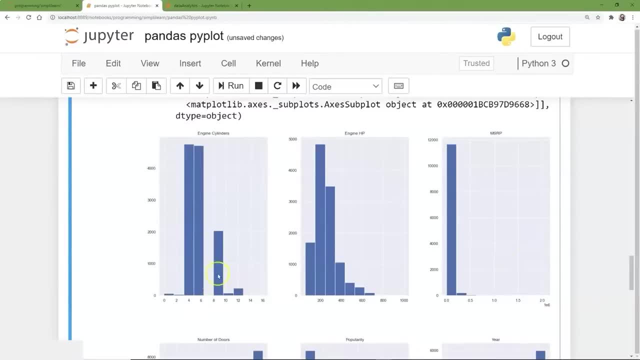 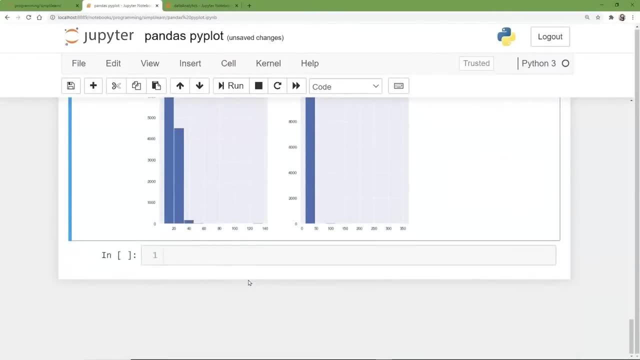 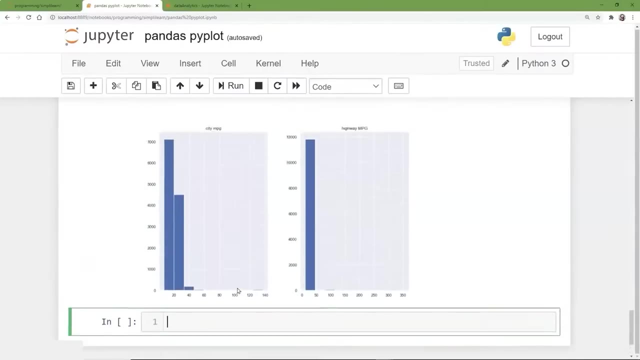 it down. So now you have how many cars with how many- whatever it is- cylinders, horsepower and how many horsepower, but it's not displaying it. You can see if you're working with your. you're going into your demo. It's really nice just to be able to type that in and boom, there it is. I can. 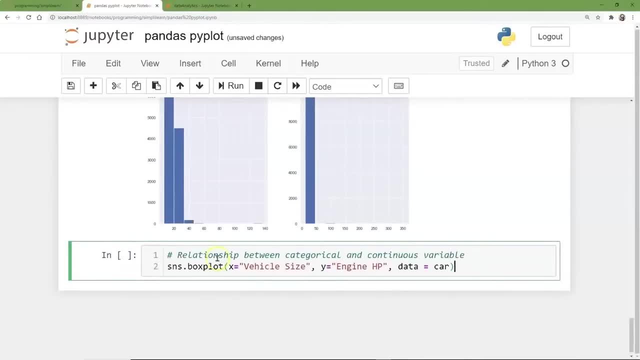 see it all the way across And we might want to zero in and use like a box plot. And this time we'll go ahead and call the Seaborn SNS box plot And we're going to go ahead and do vehicle size. 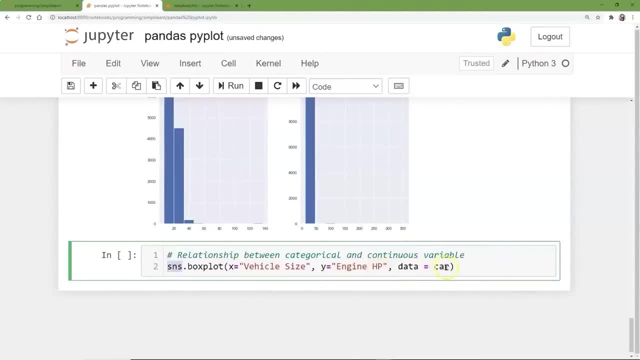 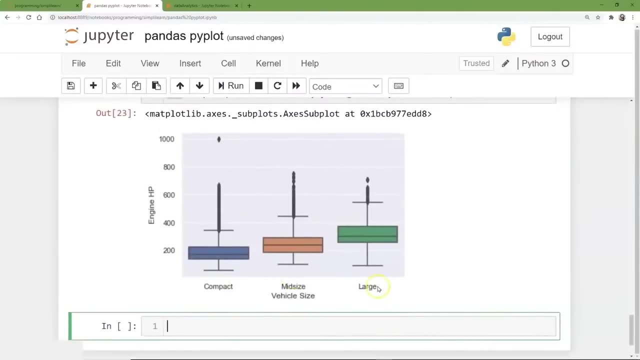 in versus engine horsepower. x, y plot comes from the car So if we run this we end up with a nice box plot. You see our midsize, compact and large. You can see the variation. There's our outlier showing. 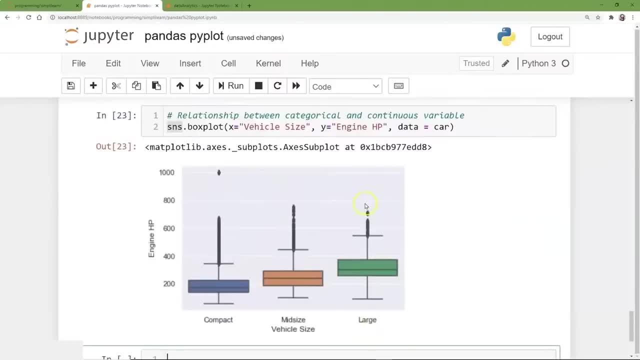 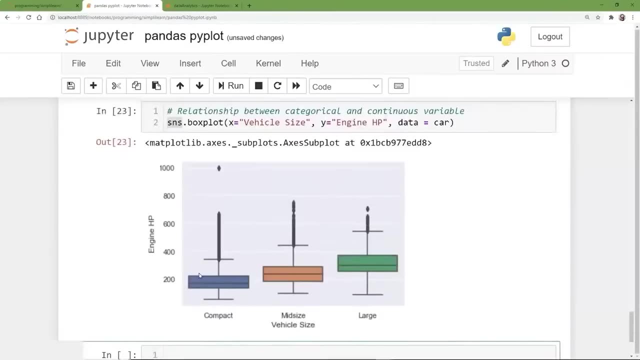 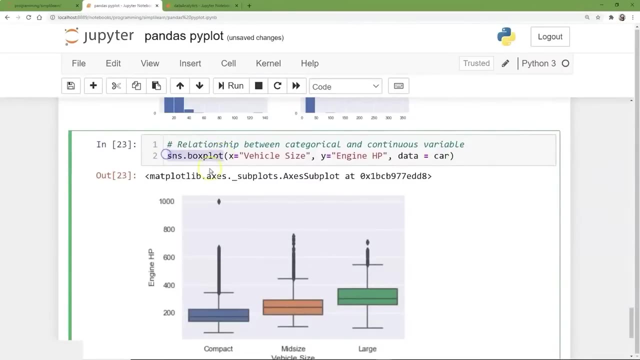 up there on the compact. That must be a high-end sports car. A large car might have a couple engines and again we have all these outliers and then your deviation on them. Very powerful and quick way to zero in on one small piece of data and display it for people who need to have it reduced to something. 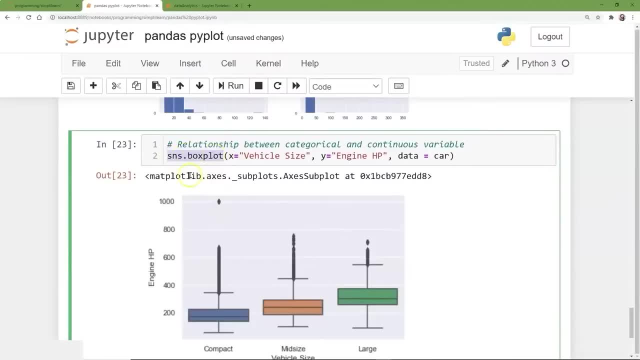 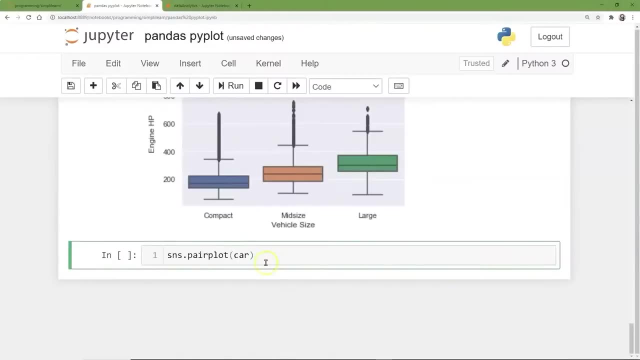 they can see and look at and understand And that's our seaborn box plot or snsboxplot. And then, if we're going to back out and we want a quick look at what they call pair plotting, we can run that and you can see with the seaborn it just 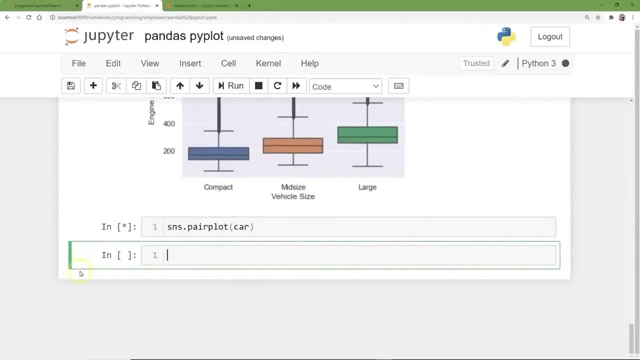 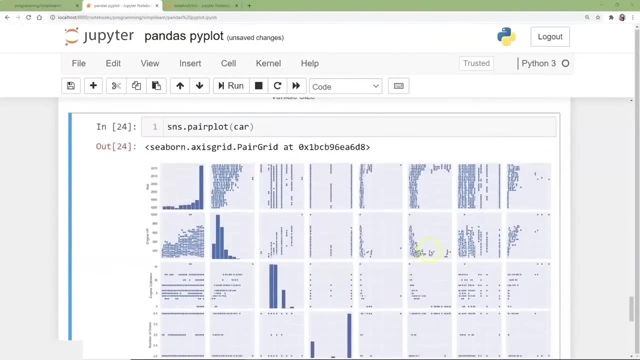 does all the work for you. It takes it just a moment for it to pull the data in and compile it and once it does, it creates a nice grid. And this grid- if you look at this one space here which is, you might not be able to see the small numbers- says engine horsepower. 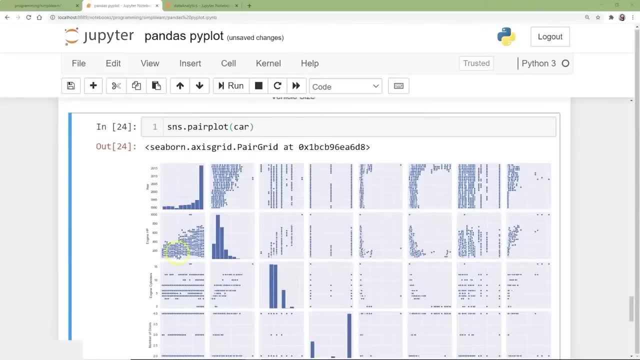 this is engine horsepower to the year it was built and it's just flipped. so everything to the right of the middle diagonal is just the rotation of what's on the left and, as you expect, the engine horsepower gets bigger and bigger and bigger as time goes on. so the the year it was built, the 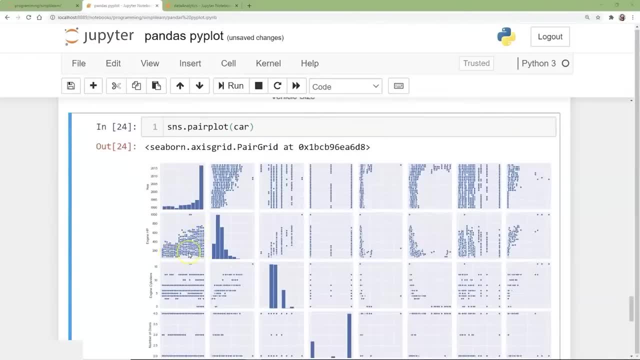 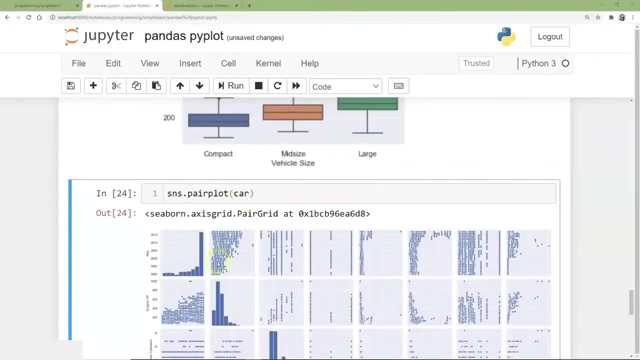 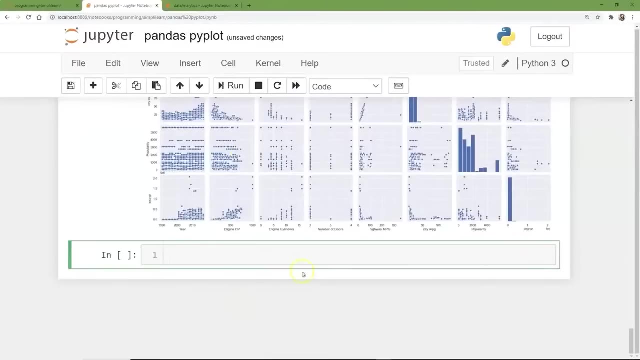 further up in the year, the more likely you are to have a heavy horsepower engine and you can quickly look at trends with our pair plot coming up and look how fast that was. that was. it took a couple you know moment to process, but right away I get a nice view of all these. 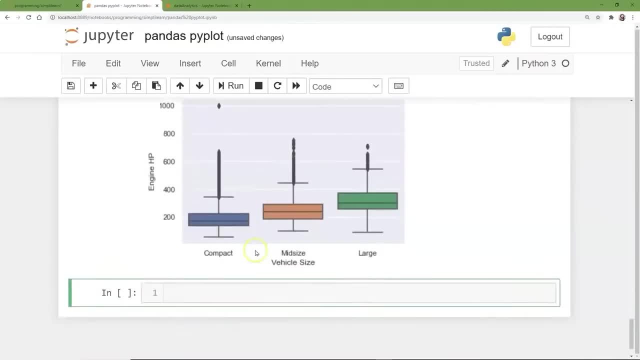 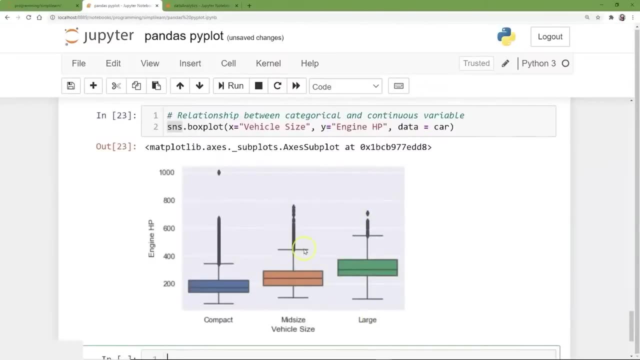 You can see the variation. There's our outlier showing up there on the compact. That must be a high-end sports car. A large car might have a couple engines and again we have all these outliers and then your deviation on them. Very powerful and quick way to. 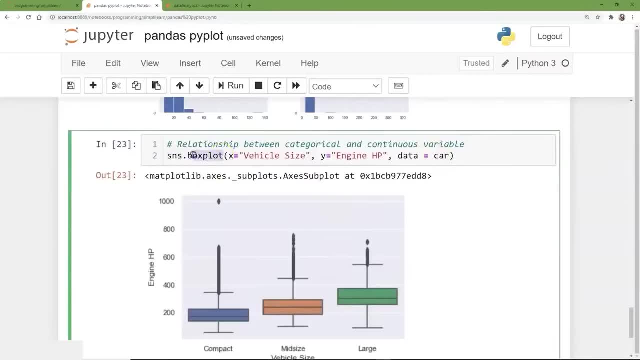 zero in on one small piece of data and display it for people who need to have it reduced to something they can see and look at and understand, And that's our Seaborn boxplot or our SNSboxplot. And then, if we're going to back out, 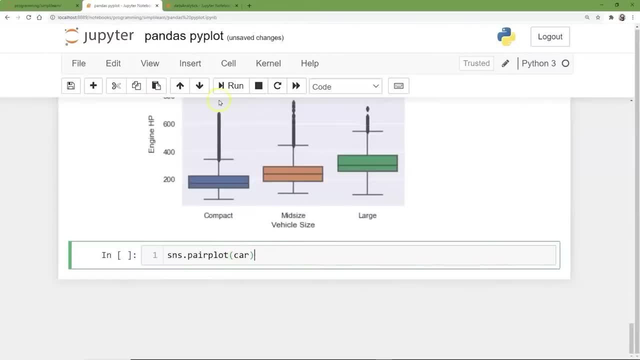 and we want a quick look at what they call pair plotting. we can run that and you can see with the Seaborn it just does all the work for you. It takes just a moment for it to pull the data in and compile it. 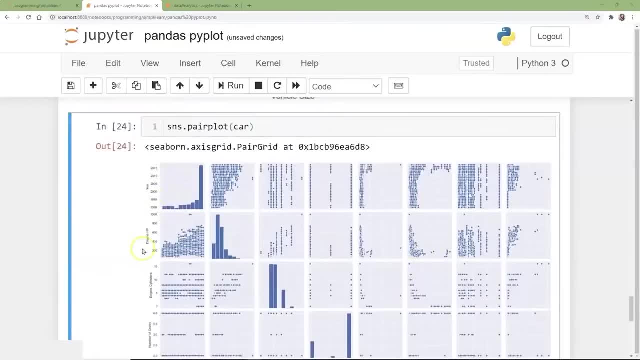 And once it does, it creates a nice grid. And this grid- if you look at this one space here you might not be able to see the small numbers- says engine horsepower. This is engine horsepower, to the year it was built And it's just flipped. 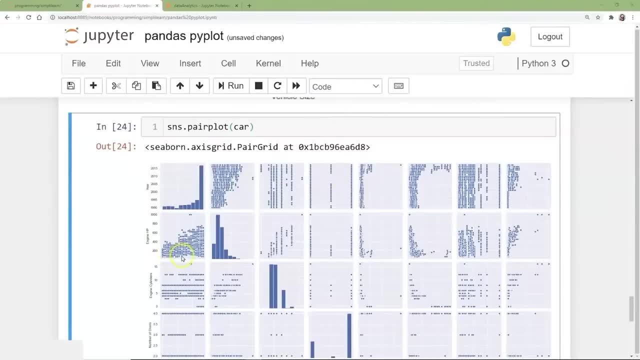 So everything to the right of the middle diagonal is just the rotation of what's on the left And, as you expect, the engine horsepower gets bigger and bigger and bigger as time goes on. So the year it was built, the further up in the year 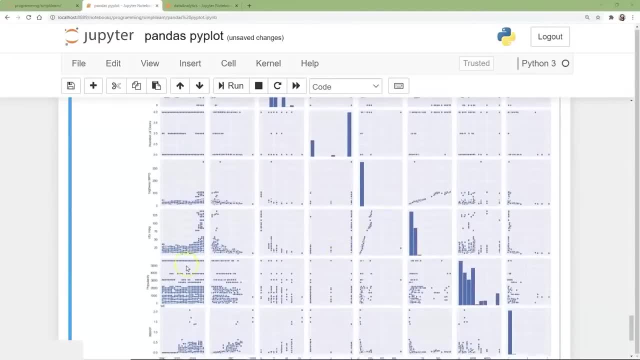 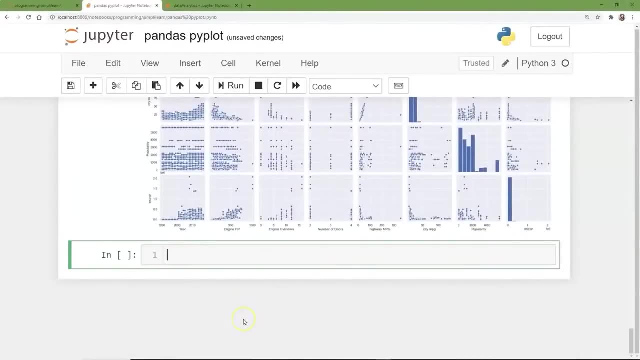 the more likely you are to have a heavy horsepower engine With our pair plot coming up And look how fast that was. It took a moment to process, But right away I get a nice view of all these different information which I can look at visually. 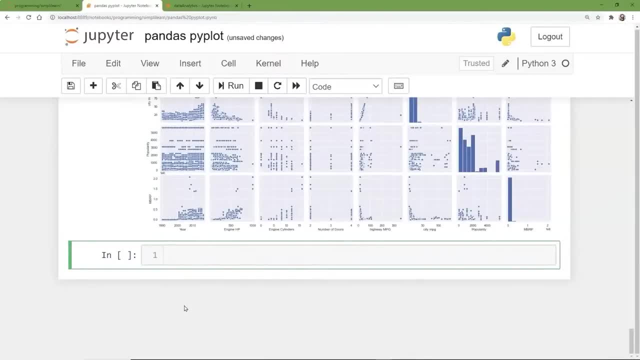 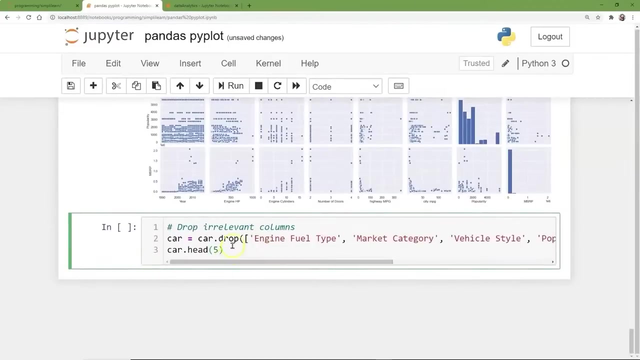 and kind of see how things group and look. Now, if I was doing a meeting, I probably wouldn't show all the data. One of the things I've learned over the years is people, myself included, love to show all our work. We were taught in school. 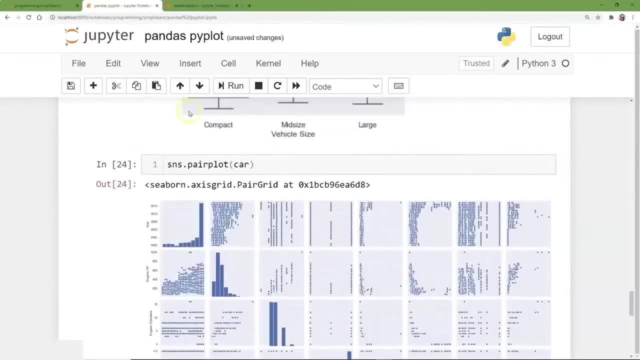 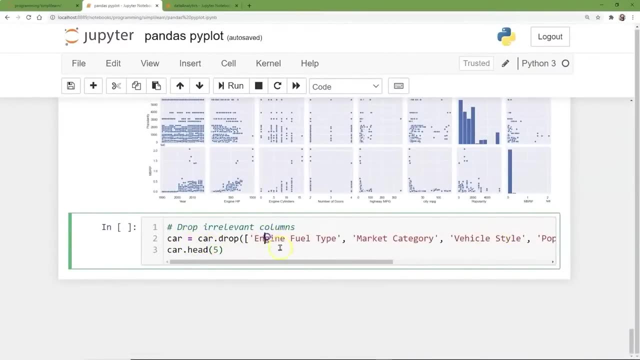 show all your work, prove what you know. The CEO doesn't want to see a huge grid of graphs, I guarantee it. So what we want to do is we want to go ahead and drop the stuff that might not be interested in. I'm not really a car person. 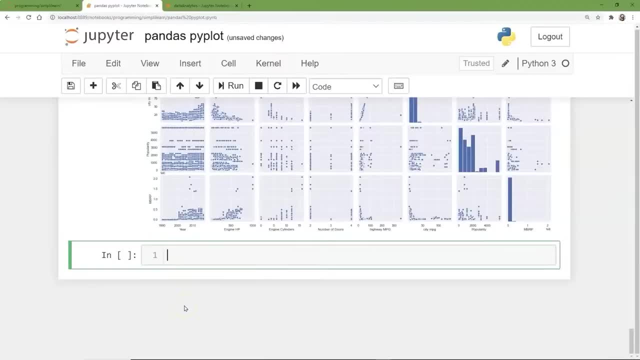 different information which I can look at visually and kind of see how things group and look. now, if I was doing a meeting I probably wouldn't show all the data. one of the things that I would look at- things I've learned over the years- is people, myself included, love to show all our work. 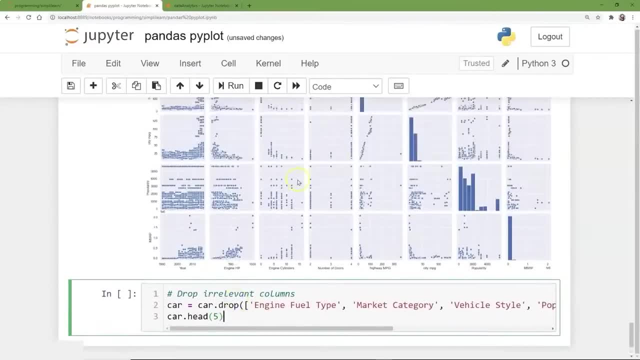 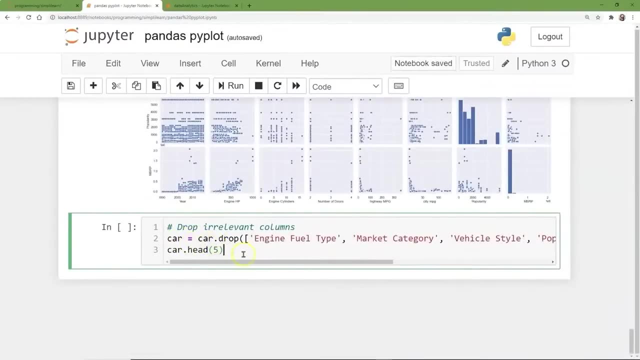 You know we were taught in school. show all your work. prove what you know. The CEO doesn't want to see a huge grid of graphs, I guarantee it. So what we want to do is we want to go ahead and drop the stuff that might not be interested in, And we're going to. I'm not really a car person. 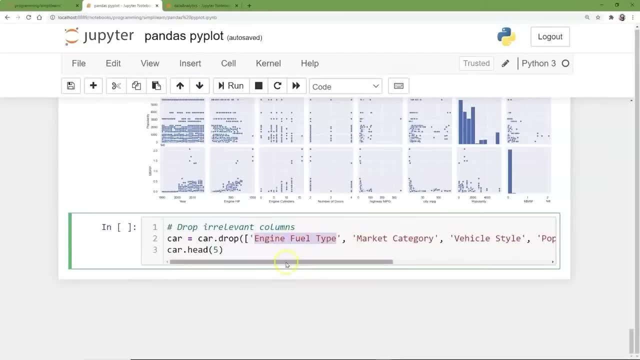 a guy in the back is obviously. So you have your engine fuel type. we're going to drop that. we're going to drop market category, vehicle style, popularity, number of doors, vehicle size And we have the axes in here. If you remember from NumPy, we have to include that, axes to make 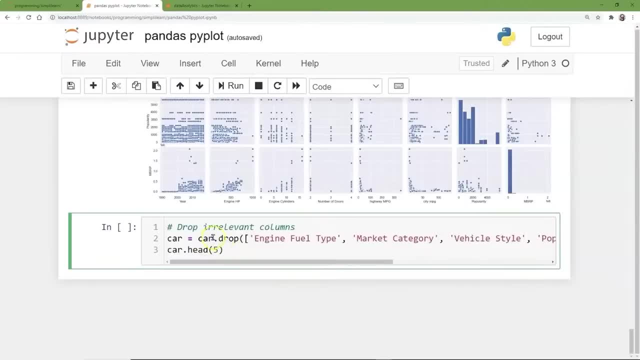 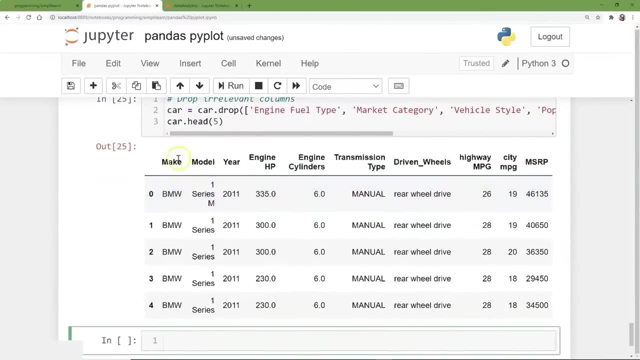 it clear what we're working on. That's also true with pandas- And then we'll look at just what it looks like from the head And you can see that we dropped out those categories And now we have the make, model year and so forth, And we took out the engine, fuel type, market category, etc. 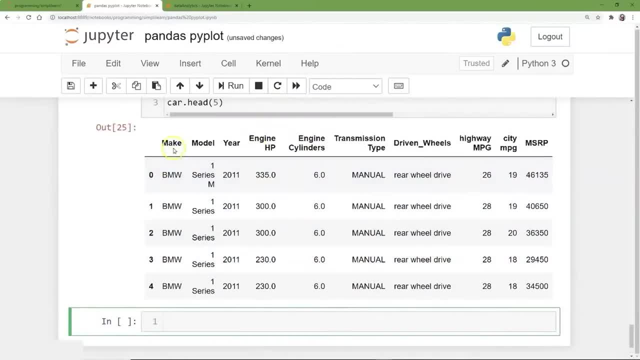 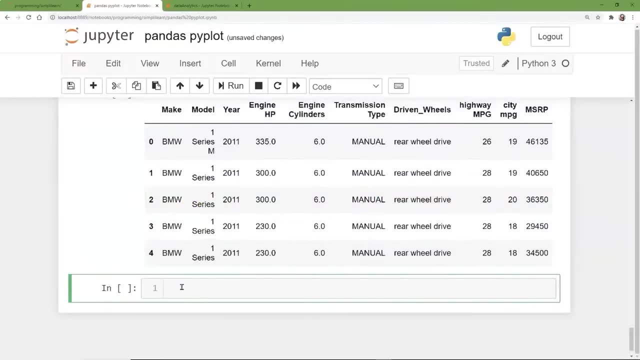 And this is look familiar to you now when you start working with pandas. I just love pandas. for this reason, Look how easy it is. It just displays it as a nice spreadsheet for you. you can just look at it and view it very easily. It's also the same kind of view. 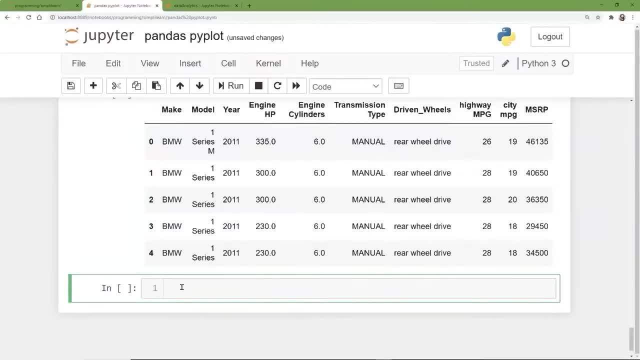 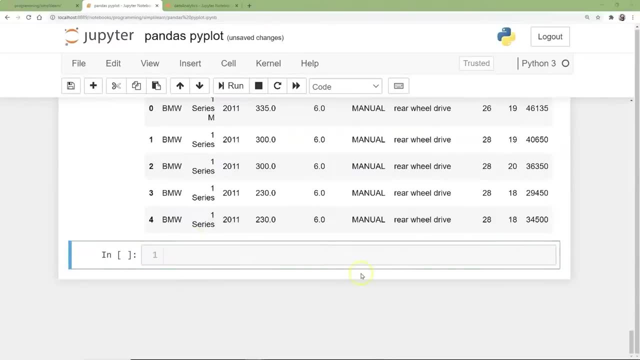 you're going to get if you're working in spark or pi spark, which is Python for Spark across big data. This is the kind of thing that they they come up with. This is why pandas is so powerful, And we may look at this and decide. we don't like these columns. 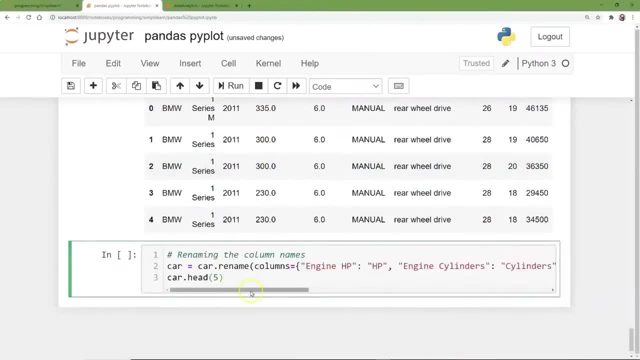 and so you can go in here and we can actually rename the columns. simple command: car equals car. rename columns equals engine horsepower equals horsepower. this is just your standard Python dictionary, so it just maps them out and, you know, instead of having like a lengthy here we had 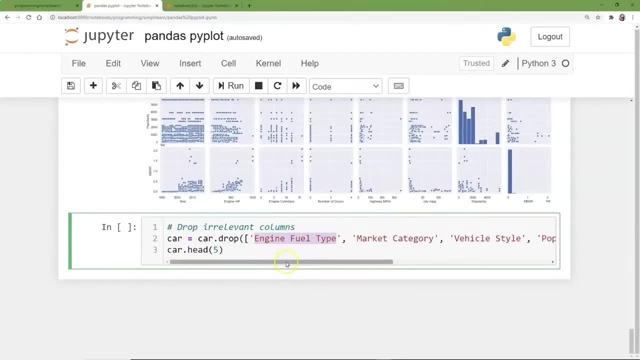 Our guy in the back is obviously. So you have your engine fuel type. we're going to drop that. We're going to drop market category, vehicle style, popularity, number of doors, vehicle size. Remember from numpy? we have to include that axis to make it clear. 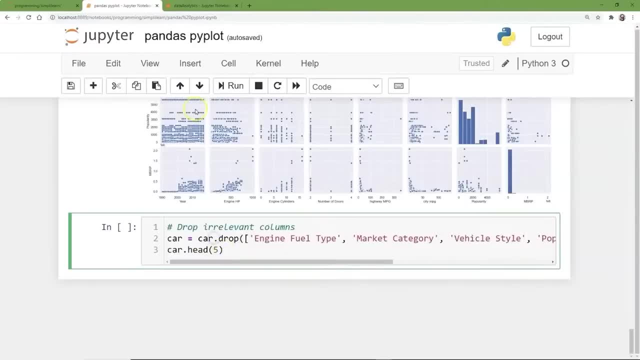 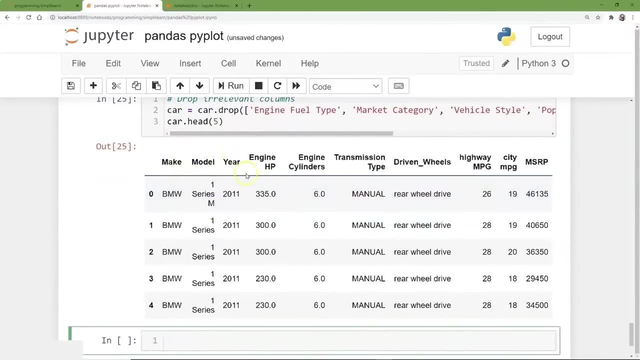 what we're working on. That's also true with pandas. Then we'll look at what it looks like from the head. You can see that we dropped out those categories and now we have the make, model year and so forth. We took out the engine fuel type. 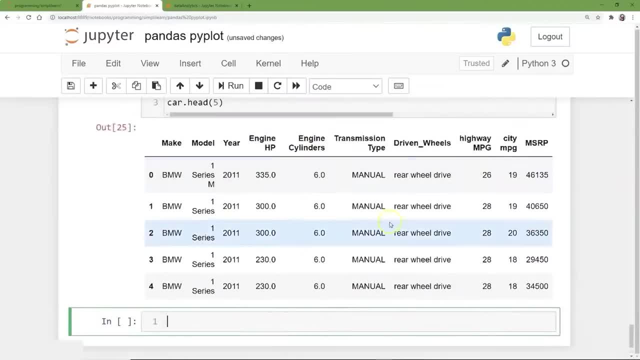 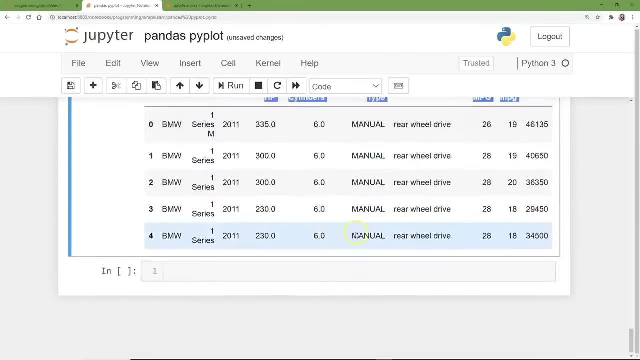 market category, etc. This should look familiar to you now When you start working with pandas. I just love pandas. for this reason, Look how easy it is. It has a nice spreadsheet for you. You can just look at it and view it very easily. 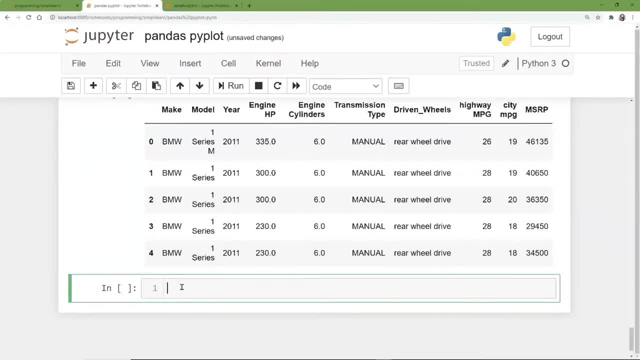 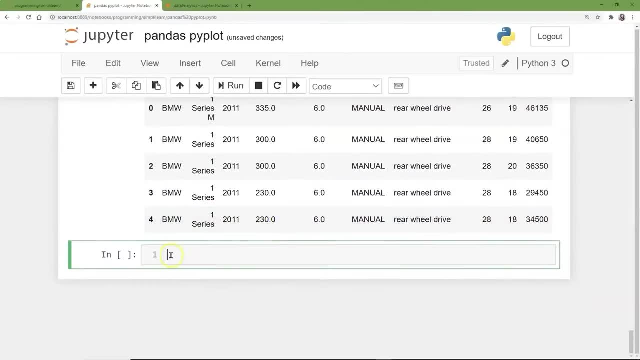 It's also the same kind of view you're going to get if you're working in Spark or PySpark, which is Python for Spark across big data. This is the kind of thing that they come up with, and this is why pandas are so powerful. 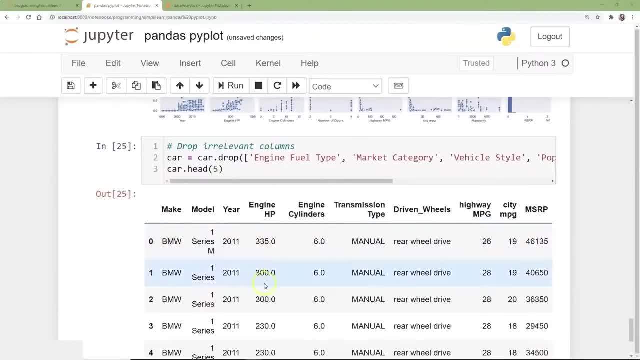 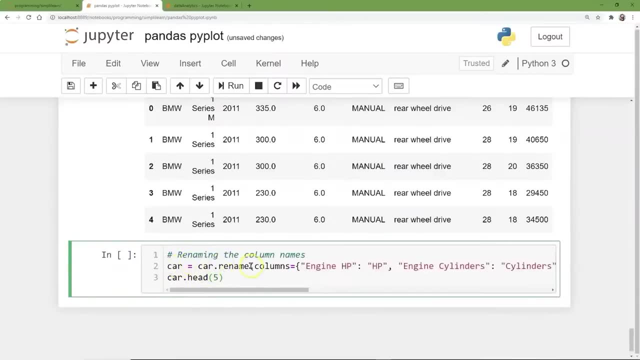 We may look at this and decide we don't like these columns. You can go in here and we can actually rename the columns. Simple command: car equals car rename Columns equals engine horsepower equals horsepower. This is just your standard Python dictionary. It just maps them out. 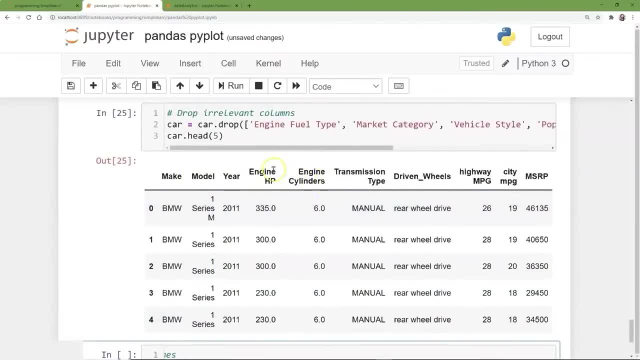 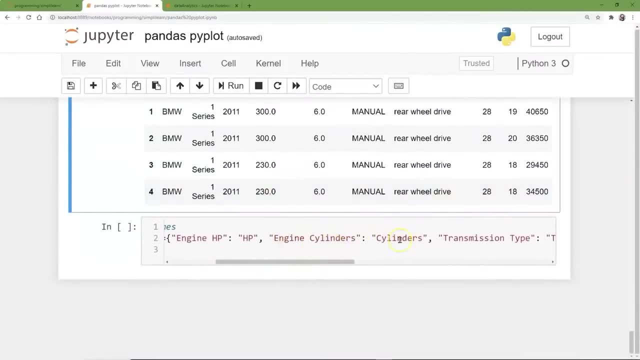 Instead of having a lengthy here. we had engine horsepower. We just want horsepower. We don't need to know it's the engine horsepower, Engine cylinders. we don't need to know that it's for the engine. There's only one thing we're describing. 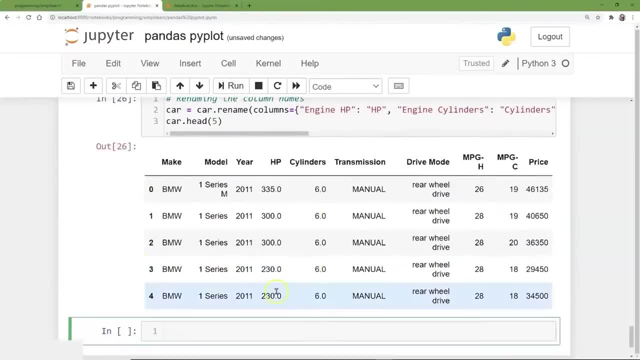 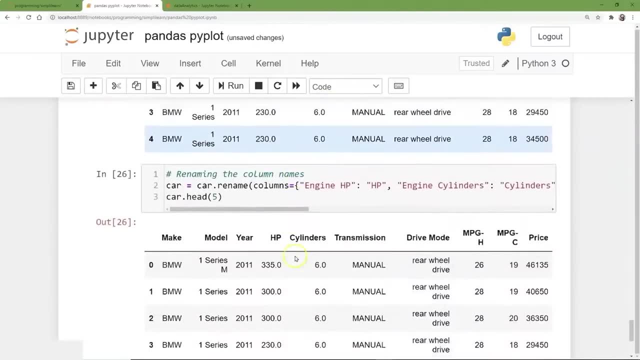 if we're talking about cars and that's cylinders, We'll go ahead and just run this Again. here's our car head. We have model year and horsepower versus model year. engine horsepower, engine cylinders and just cylinders. Again, we want to keep reducing this. 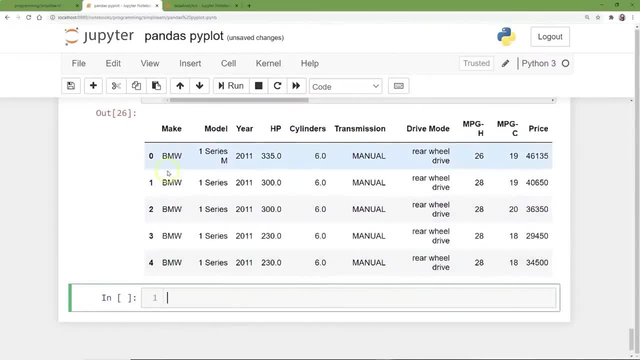 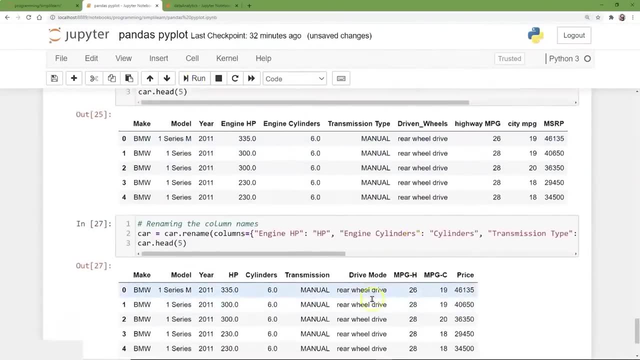 so it's more and more readable. The more readable you get it, the better. Of course, we can also adjust the size a little bit so that when it prints out, instead of splitting it on two lines, we get a single line. 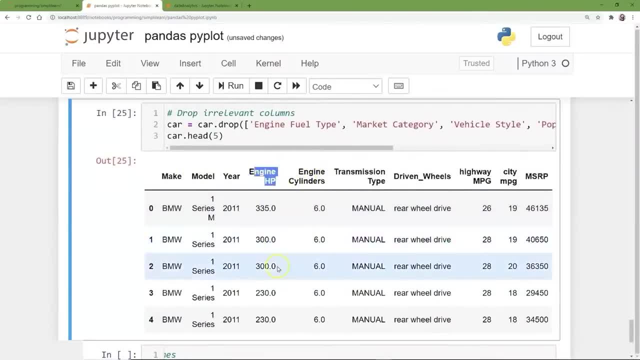 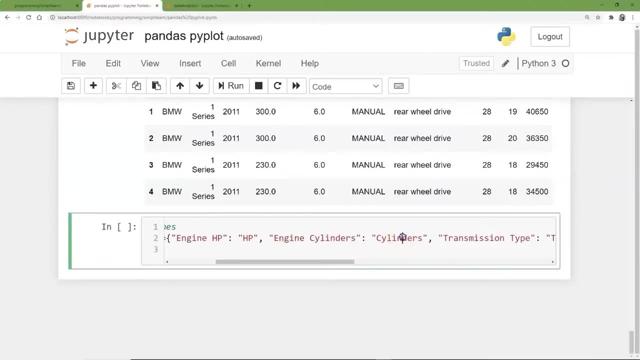 engine horsepower, we just want horsepower. we don't need to know it's the engine horsepower, engine cylinders. we don't need to know that it's for the engine, because there's only one thing we're describing if we're talking about cars, and that's cylinders, and we'll go ahead and just run this and again, here's our car head and you can see. 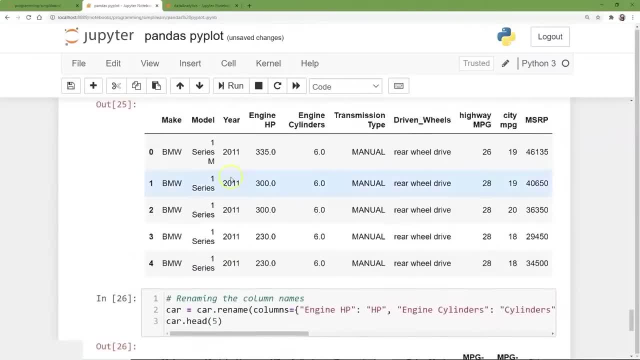 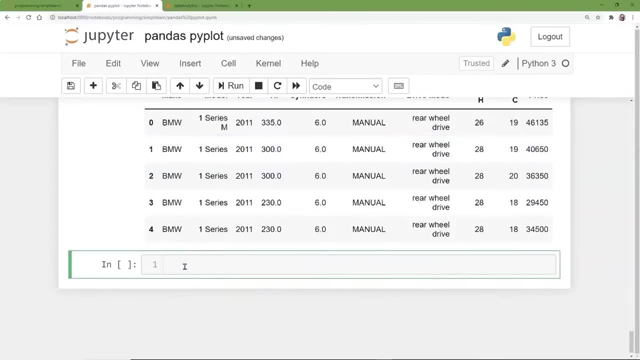 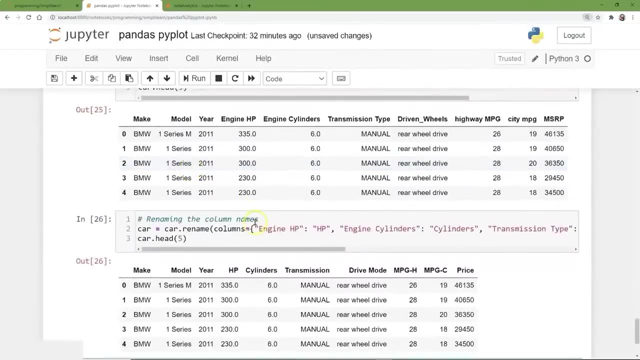 how that changed. we have model year and horsepower versus model year engine, horsepower, engine cylinders and just cylinders. again, we want to keep reducing this, so it's more and more readable. the more readable you get it, the better, and of course we can also adjust the size a. 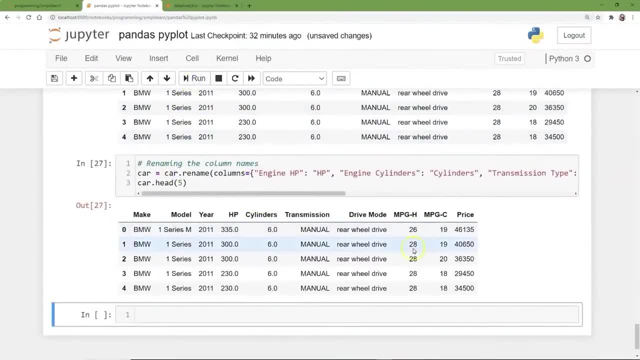 little bit so that when it prints out, instead of splitting it on two lines, we can also adjust the size a little bit, so that, when it prints out, instead of splitting it on two lines, we can also adjust the size a little bit so that, when it prints out, instead of splitting it on two lines. 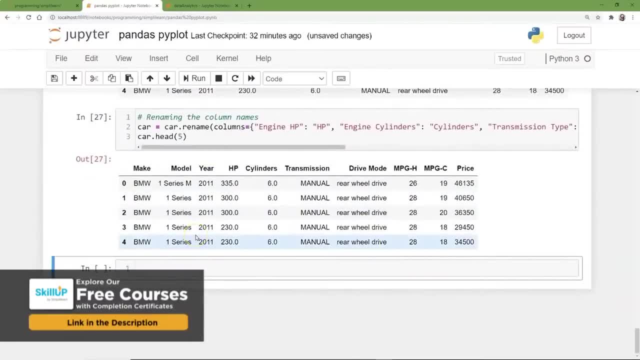 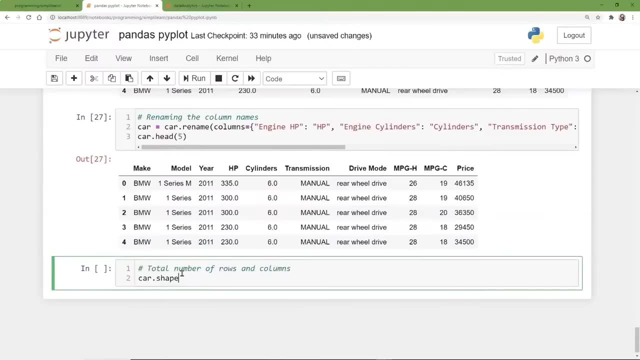 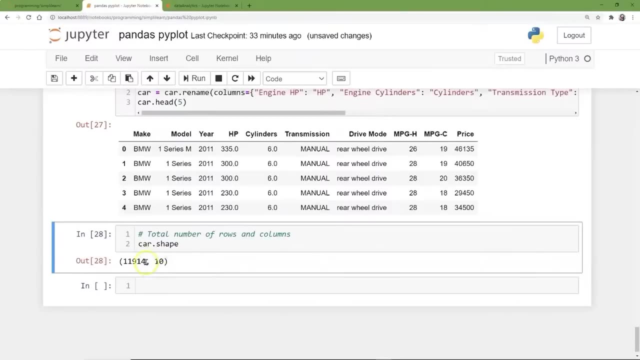 we get like a single line. we can do that also. that's just your control mouse up or plus sign you use in chrome. that's a chrome command and if you remember from numpy we had shape. well, pandas works the same way. we can look at the shape of the data. so we now have 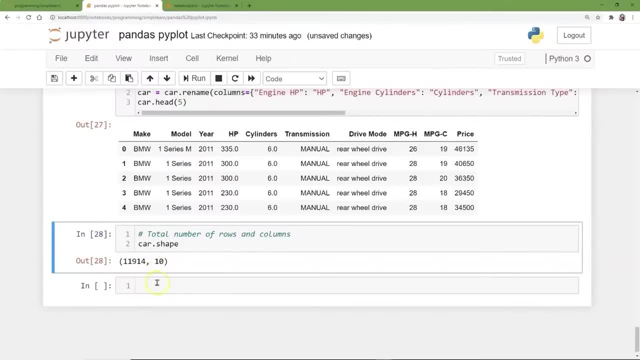 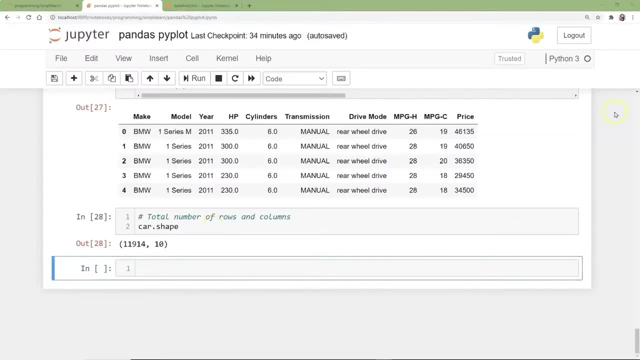 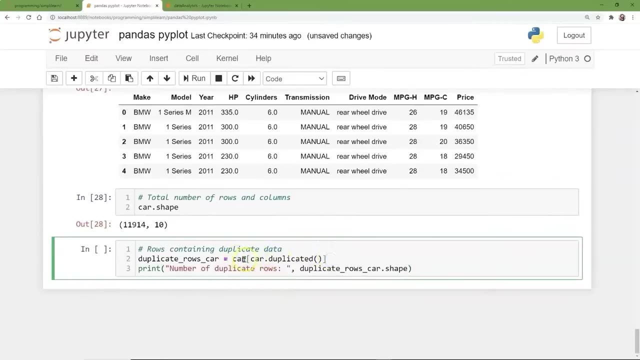 11,914 rows and 10 columns. so you see some similarities. because pandas is built on numpy and questions that come up just like we did in numpy. we might want to know duplicate rows and so we can do car and look at this switch. here we're doing a selection. 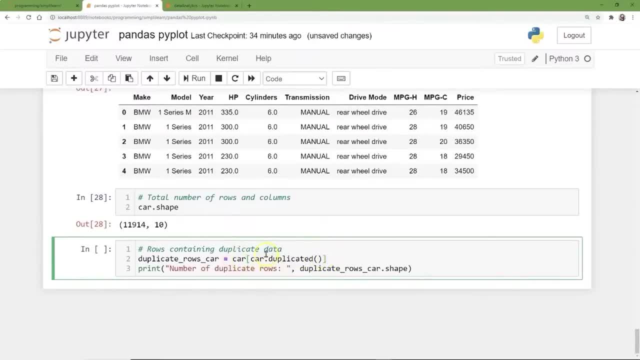 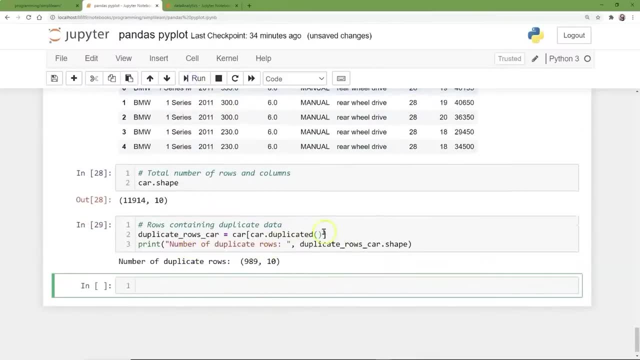 this is a pandas selection with the brackets, but we want to select it based on car dot duplicated. so how many duplicates on there? so it's starting to look a little bit different. as far as how we access some of the data on here, this can be a logical statement. 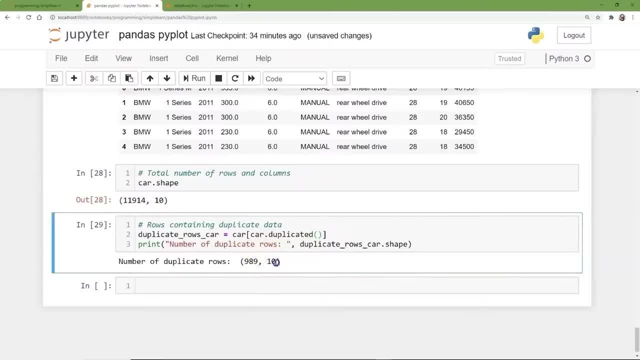 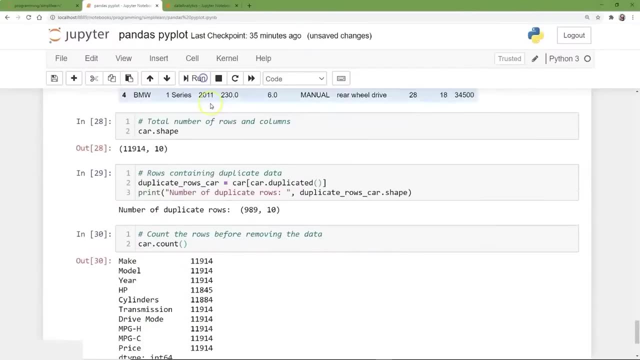 and we get the number of duplicate rows, we have 989 rows by 10 columns again, and this is one of those troubleshooting things that we end up doing a lot more than we really feel like we should. we might go ahead and do like a car count. 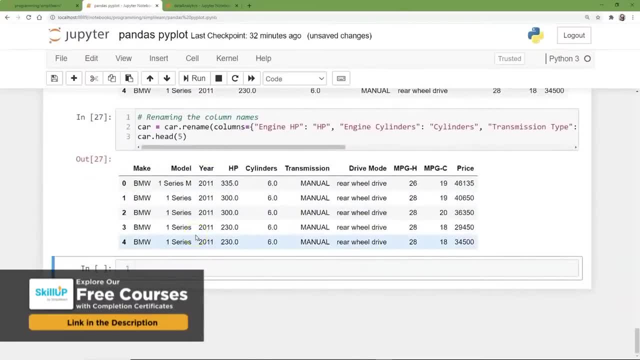 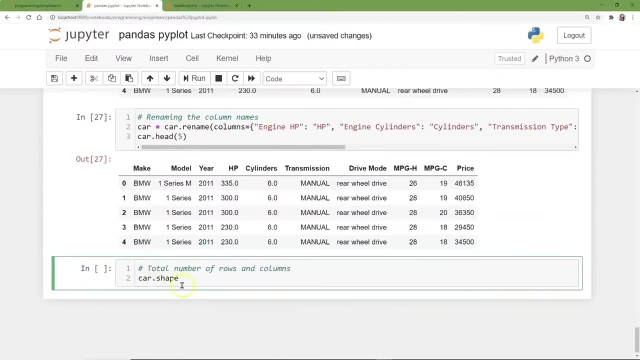 We can do that also. That's just your control mouse up or plus sign you use in Chrome. That's a Chrome command. If you remember from NumPy, we had shape Pandas works the same way. We can look at the shape of the data. 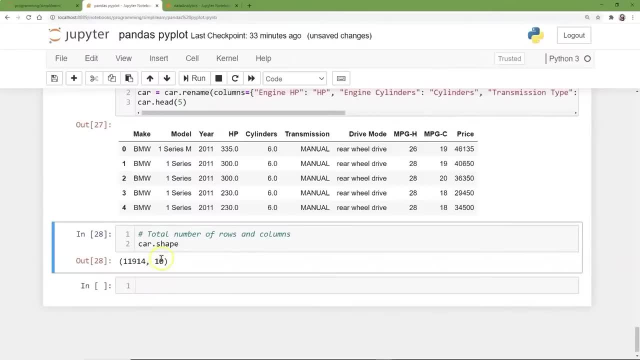 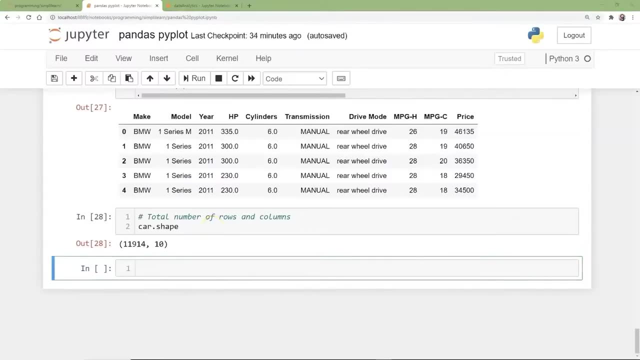 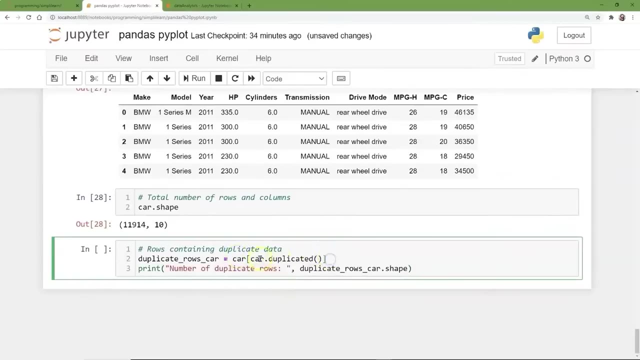 We now have 11,914 rows and 10 columns. You see some similarities because Pandas is built on NumPy- Questions that come up just like we did in NumPy. we might want to know duplicate rows. We can do car. 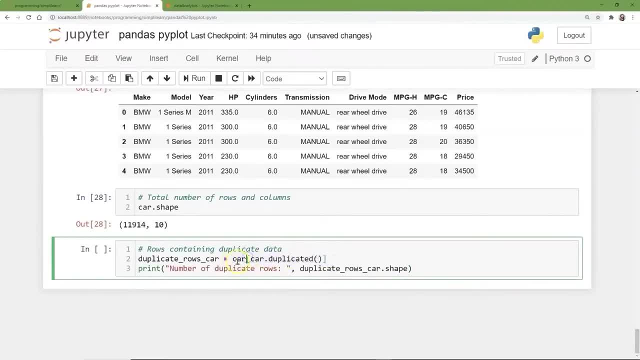 Look at this switch. here We're doing a selection, Pandas selection with the brackets. We want to select it based on carduplicated- How many duplicates on there? It's starting to look a little bit different as far as how we access some of the data. 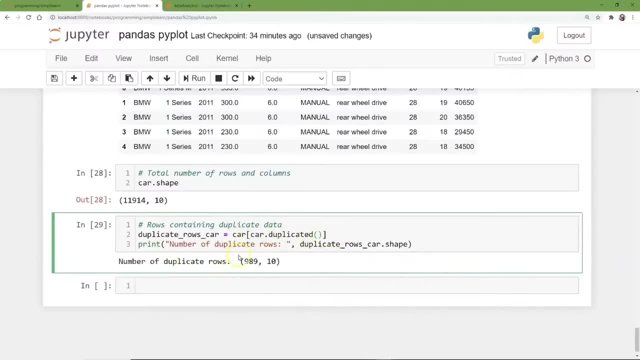 on here. This can be a logical statement. We get the number of duplicate rows. We have 989 rows by 10 columns again. This is one of those troubleshooting things that we end up doing a lot more than we really feel like we should. 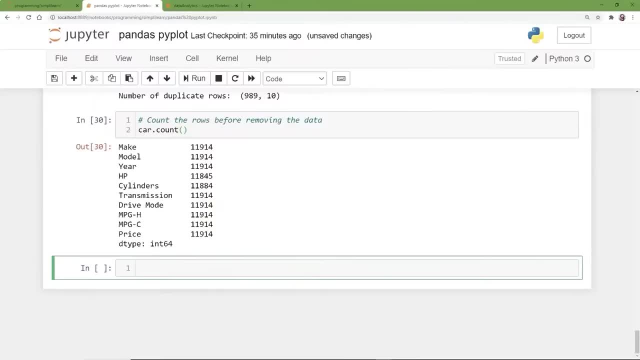 We might go ahead and do a car count Just to see how many rows we're dealing with. Then, right after that, we might want to go ahead and say: let's drop duplicates. Remember, we did all the duplicates on there. Car equals cardrop duplicates. 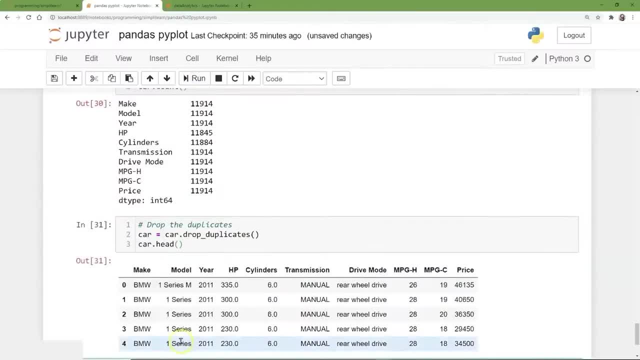 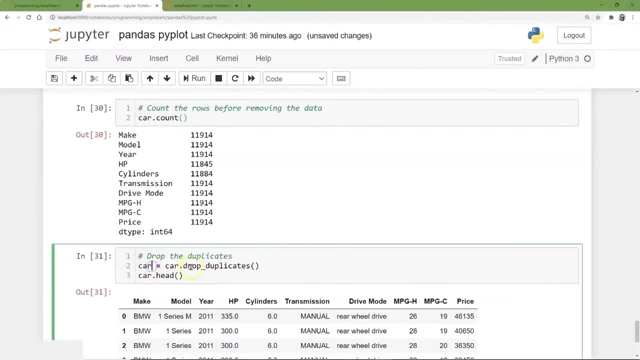 Then we can print the head again. We'll just do car head here. You can see the data on there looks the same as before. Just note that we did car equals cardrop duplicates. There are commands in here where you can do where it changes the actual. 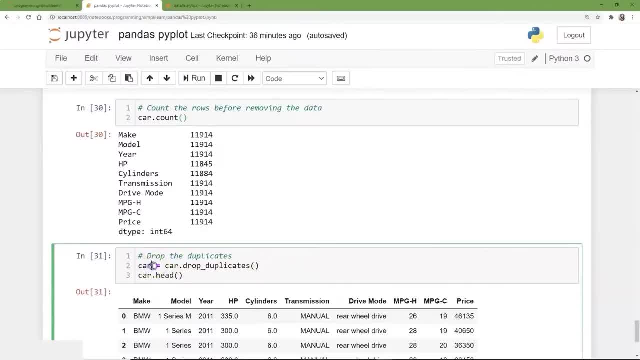 value. It works on some of them and not on others, depending on what you're doing. By default, it always returns a copy. When we do this, we're reassigning it to car. You can see it's the same header, but we want to go ahead and do count. 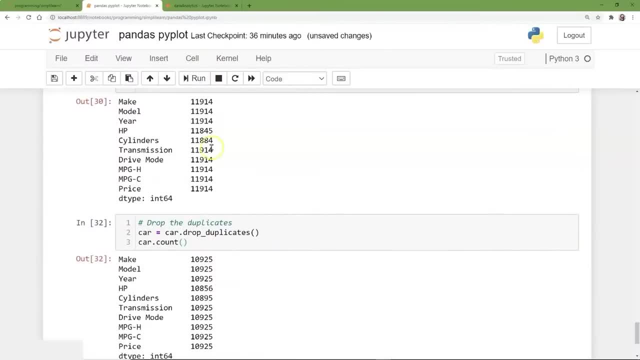 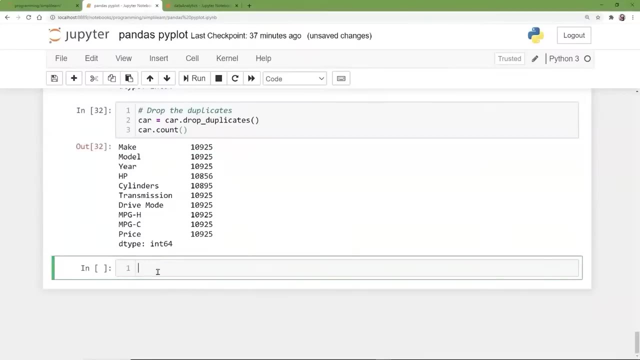 See how the count changes. Let's go ahead and run this. You can see here, instead of 11914 we have 10925.. We've removed about 100 cars that were duplicated Just slightly under 100.. Then, as we're prepping our data, 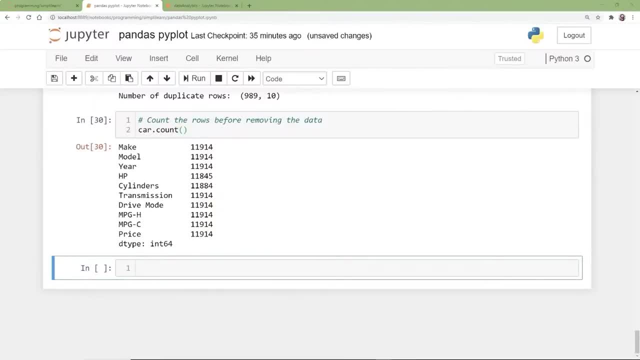 just to see how many rows we're dealing with, and then right after that we might want to go ahead and say, hey, let's drop duplicates. so remember, we did all the duplicates on there, so car equals car dot. drop duplicates, and then we can print the head again. 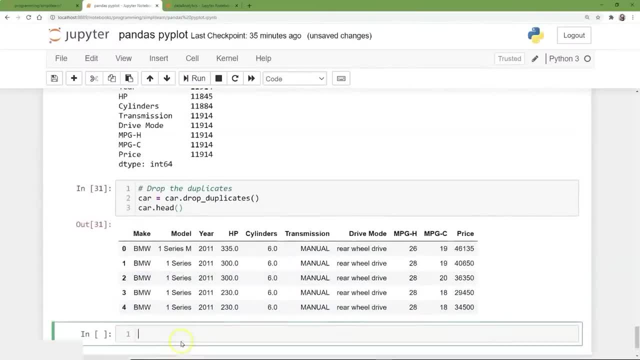 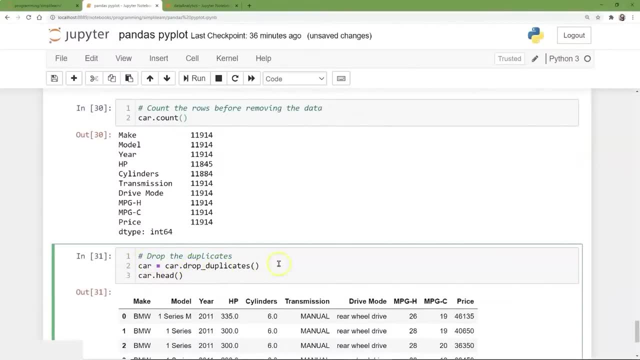 we'll just do car head here and you can see the data on there looks the same as before and just note that we did car equals car dot duplicates. there are commands in here where you can do where it changes the actual value and it works on some of them and not on others, depending on what you're doing. 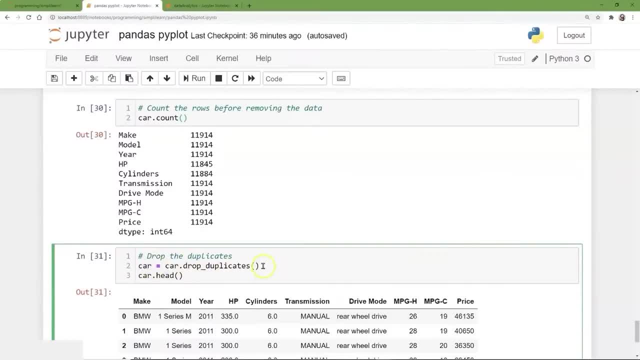 but by default it always returns a copy. so when we do this we're reassigning it to car and you can see it's the same header. but we want to go ahead and do count and see how the count changes. let's go ahead and run this. 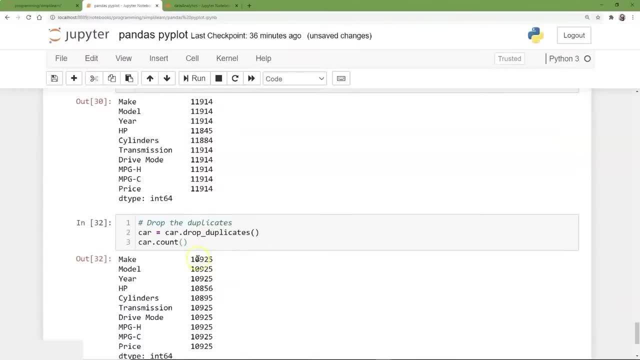 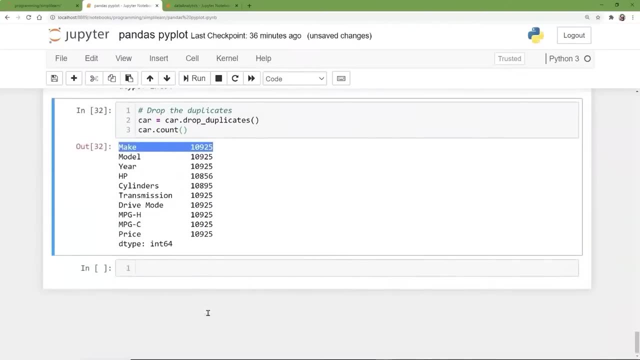 and you can see here, instead of 11,, 9,, 14, we have 10,925. so we've removed about 100 cars that were duplicated just slightly under 100 there. and then, as we're prepping our data, we might want to know: car is null. 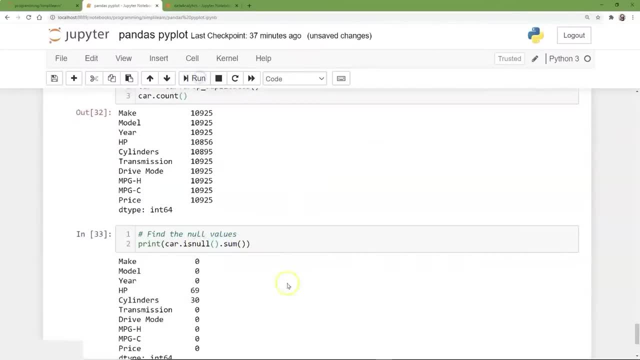 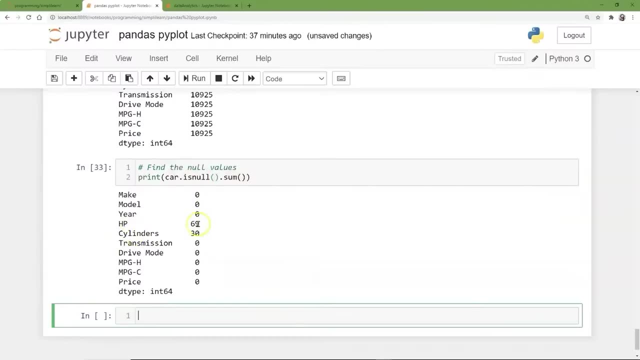 so it's going to count the values of null and then we want to sum that up, and when we do that we do the car is null. function dot sum. we end up with HP, the horsepower is 69, have null values and cylinders have null values. now, if you don't put the sum at the end, 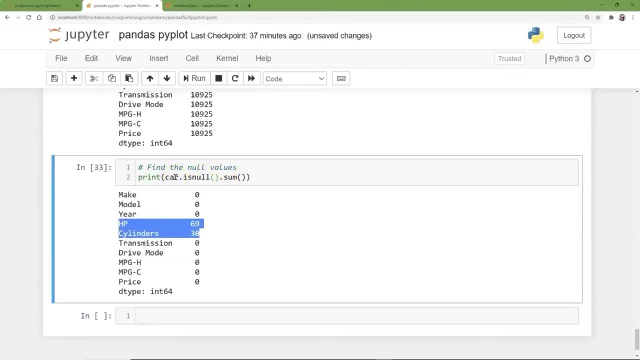 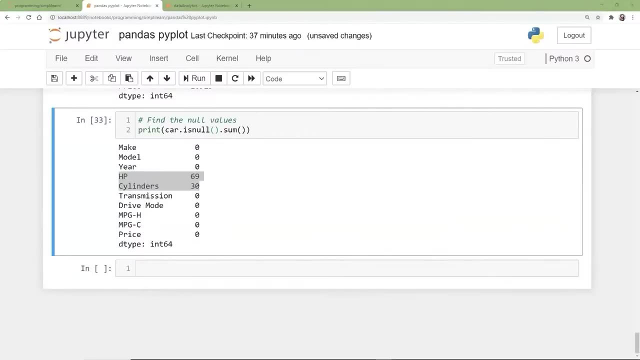 it's just going to return a mask with the true false of: is it null or is it not by zero and one. so you're summing up the ones underneath each column and this, of course. then you have to decide what you're going to do with the null values. 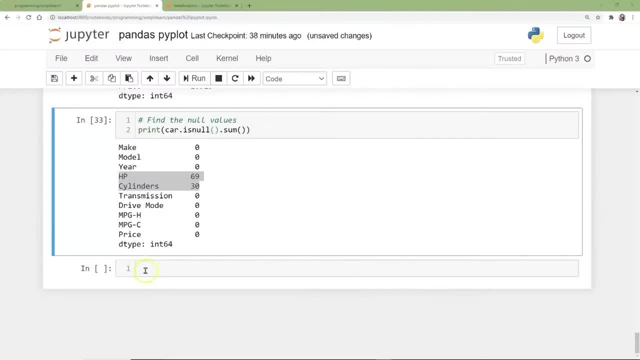 there's a lot of different options. it might be that you need to put in the average or means. maybe you want to put in the median value. there's a lot of different ways to fill it. usually when you first start out with the data- a lot of them- you just drop your null values. 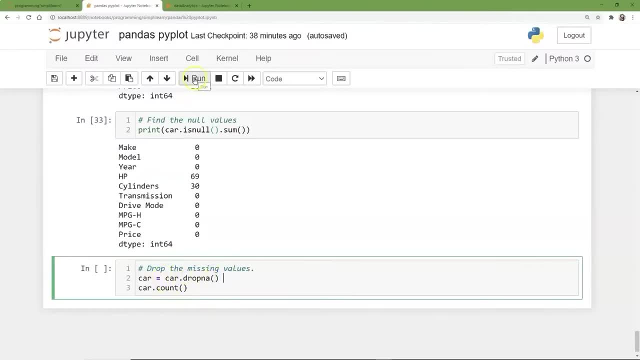 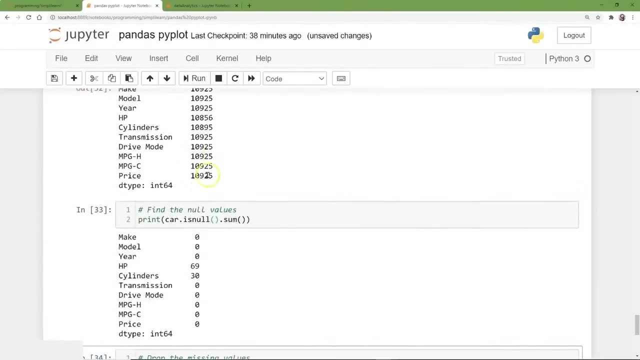 and you can see here: car dot drop NA, which is equal to all, and then we're going to go ahead and count it and you can see that we've dropped almost another 100 values. so from 10,925 to 10,827, maybe 75 or so values. 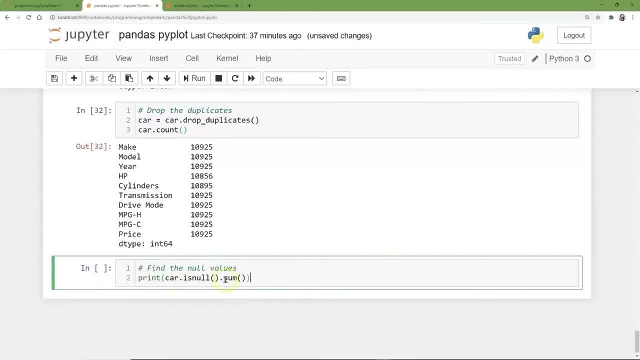 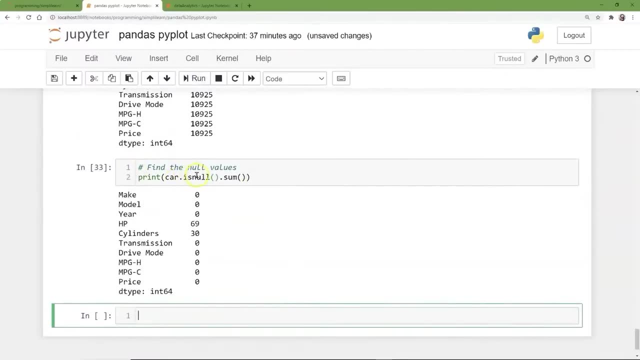 we might want to know. car is null. It's going to count the values of null and then we want to sum that up. When we do that, we do the car is null. function dot sum. We end up with HP, the horsepower is 69, have null values and 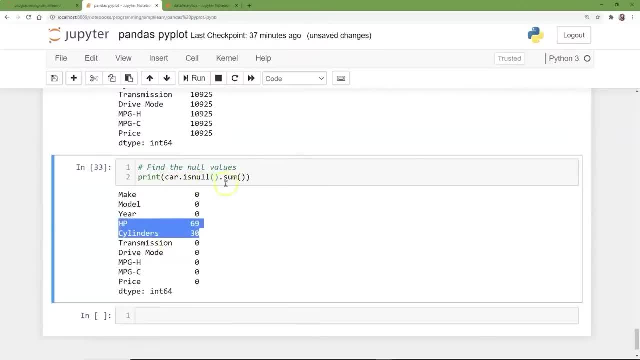 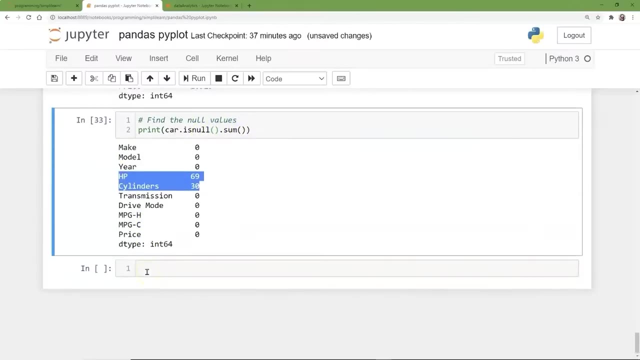 cylinders have null values. Now, if you don't put the sum at the end, it's just going to return a mask with the true false of: is it null or is it not, by 0 and 1.. You're summing up the ones underneath each column. 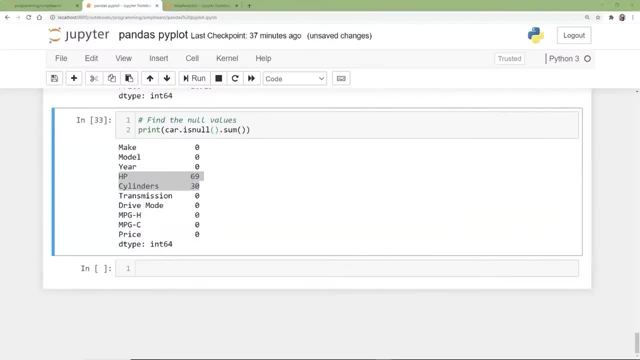 This, of course. then you have to decide what you're going to do with the null values. There's a lot of different options. It might be that you need to put in the average or means. Maybe you want to put in the median value. 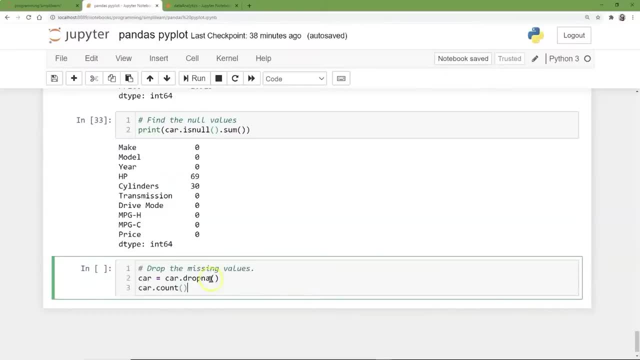 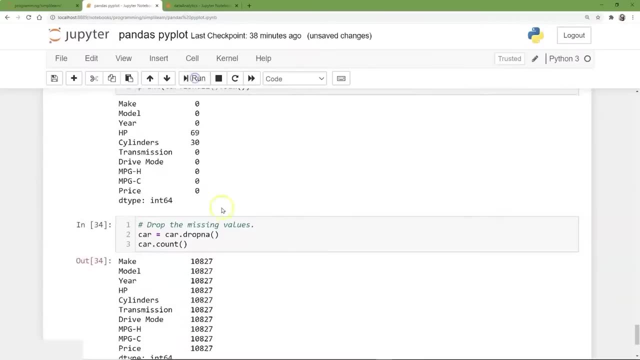 There's a lot of different ways to fill it. Usually, when you first start out with the data- a lot of them- you just draw and drop your null values. You can see here: car dot, drop NA, which is equal to all, and then we're going to go ahead and count it and you can see. 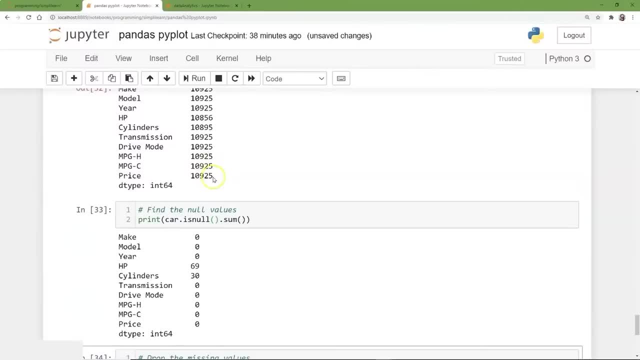 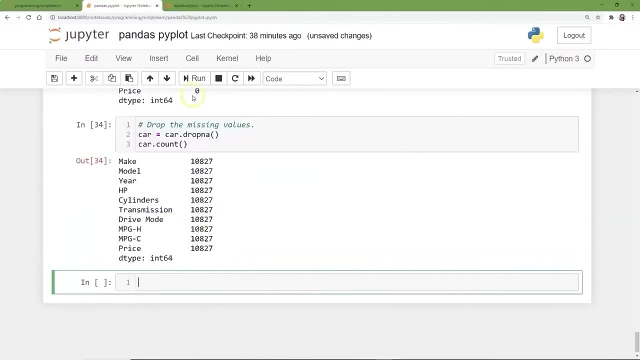 that we've dropped almost another 100 values, So from 10, 19, 25 to 10, 8, 27.. Maybe 75 or so values. This is really a big part of cleaning data. You need to know how to get. 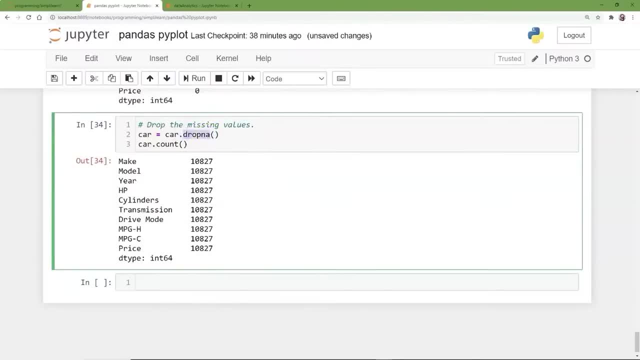 rid of your null values, or at least count them and what to do with them. Of course, if we go back to counting our null values, we should now have null null values. There we go And you'll see there's zero null values. I don't know how many times I've been running a model. 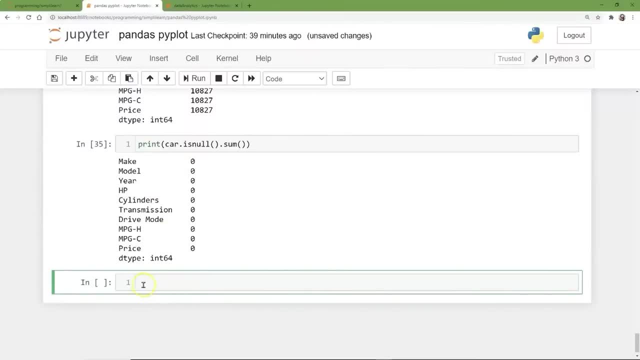 that doesn't take null values and it crashes. and I just sit there and look at it trying to get: why did that crash? It should have worked. It's because I forgot to remove the null values, So we've been jumping around a lot. 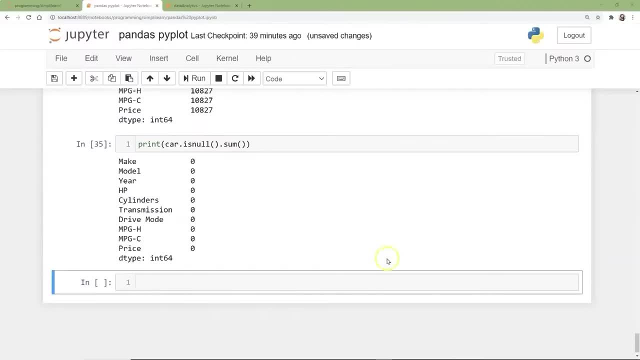 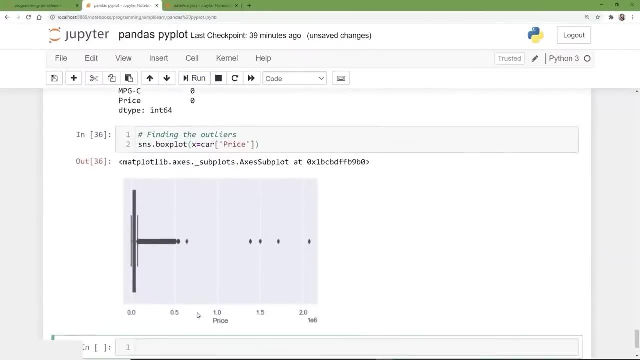 We're going to go back to finding outliers And let's go ahead and bring that back into our Seaborn And, if you remember, we did a box plot earlier. This time we're going to do a box plot, just on the price. 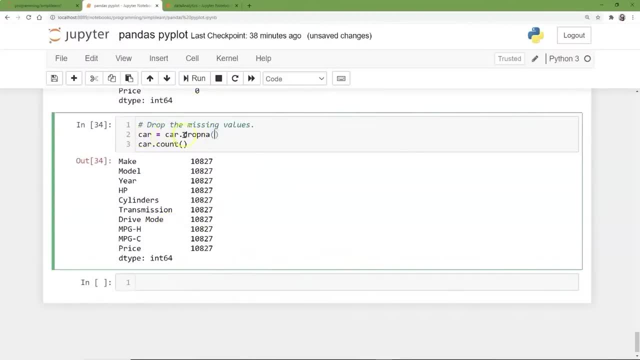 so we've cleaned it. this is really a big part of cleaning data. you need to know how to get rid of your null values, or at least count them, and what to do with them. and, of course, if we go back to counting our null values, we should now have null null values. 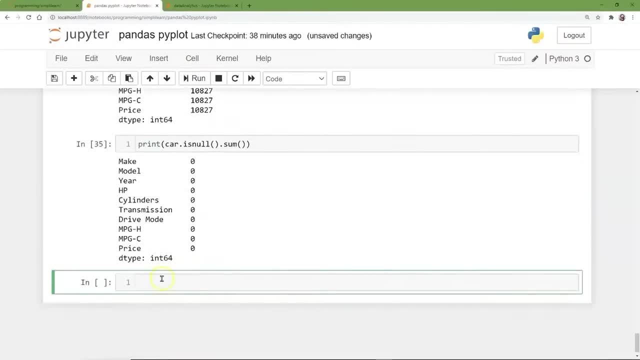 there we go and you'll see there's zero null values. I don't know how many times I've been running a model that doesn't take null values and it crashes. and I just sit there and look at it trying to get. why did that crash? 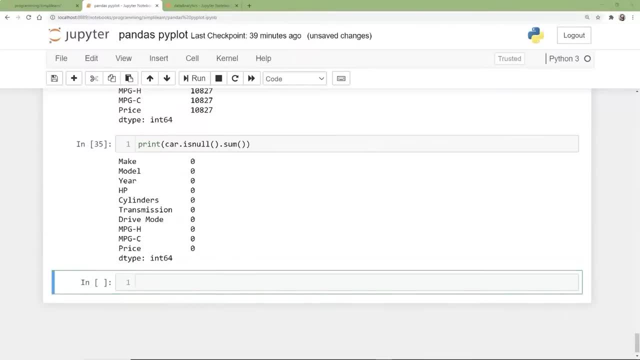 it's because I forgot to remove the null values, so we've been jumping around a lot. we're going to go back to finding outliers and let's go ahead and bring that back into our Seaborn. and if you remember, we did a box plot earlier. 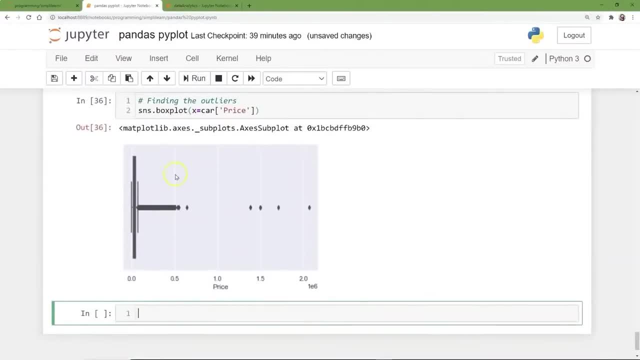 this time we're going to do a box plot just on the price and you can see here our price value and we have the deviation with the two thinner bars on each side of the main value and then as we get up here we have all these outliers. 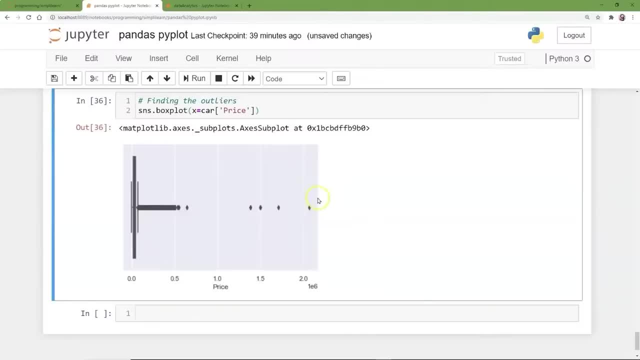 in fact, we have one way out here. that's probably a really expensive high-end car is what we're looking at. if you were doing fraud analysis, you would be jumping on all over these outliers. why are these deviation from the standard? what are these people doing? 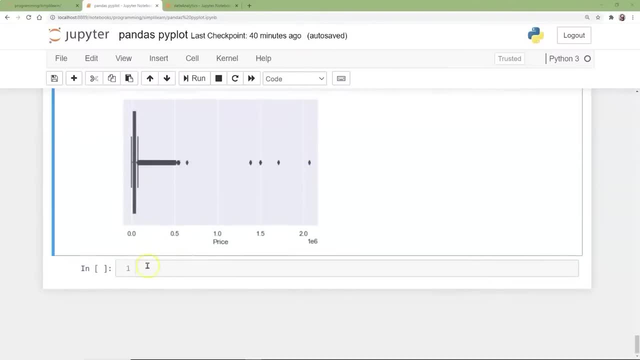 again. this is probably, like I said, a really high-end, expensive car out here. that's what we're looking at and we can also look at the box plot for the horsepower. we'll put that in down here and run that and you can see again. here's our horsepower. 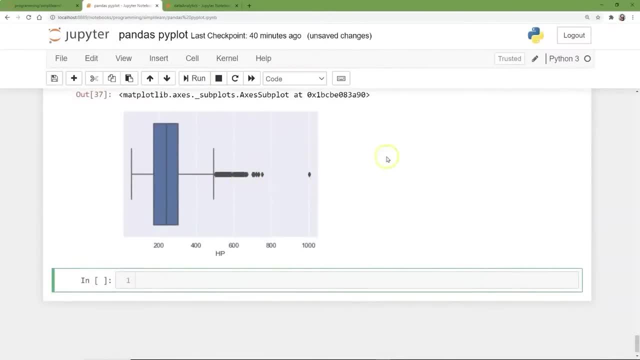 and it just jumps. and there's these really odd huge muscle cars out here that are outliers, and we're going to jump into making this a little bit more. as you start displaying your data or your information to your shareholders, we're going to look at plotting a histogram. 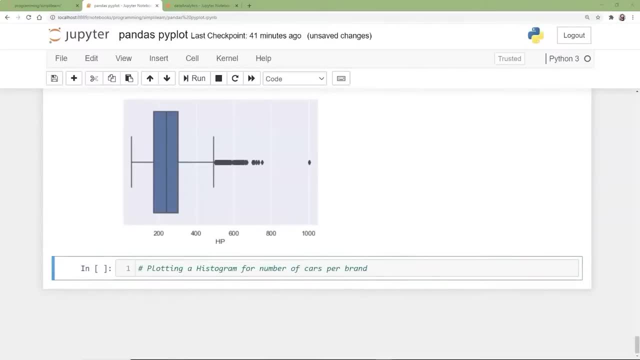 for the number of cars per brand, and the first thing we want to go ahead and do is we have with our car. let me go back over here. here we go. we have our make, value counts, largest plot and we want to do a kind equals bar figure, size, ten, five. 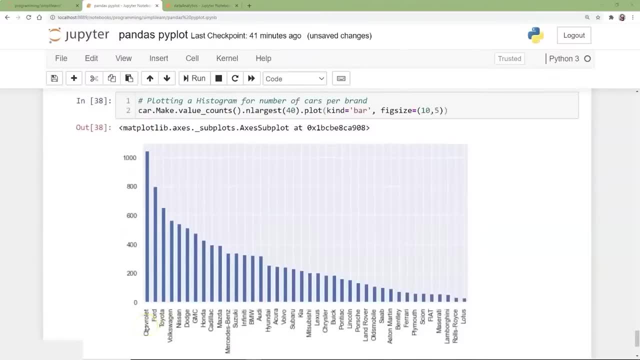 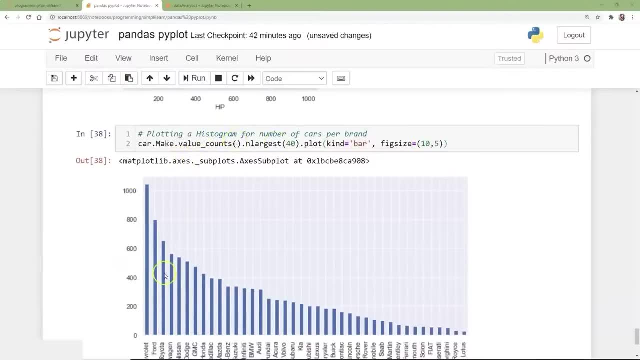 and right off the bat we jump up here and we see Chevrolet. it's going against what was it? it's figure racing. the value counts and we want the largest value. so here's our value counts and compared to what the different cars are, Chevrolet puts out a lot of different kinds of cars. 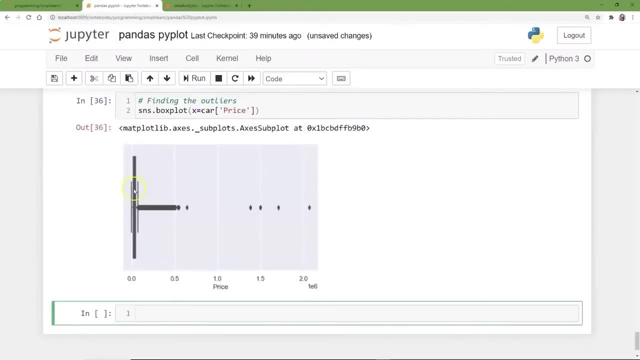 And you can see here our price value and we have the deviation with the two thinner bars on each side of the main value, And then, as we get up here, we have all these outliers. In fact, we have one way out here. that's probably a really 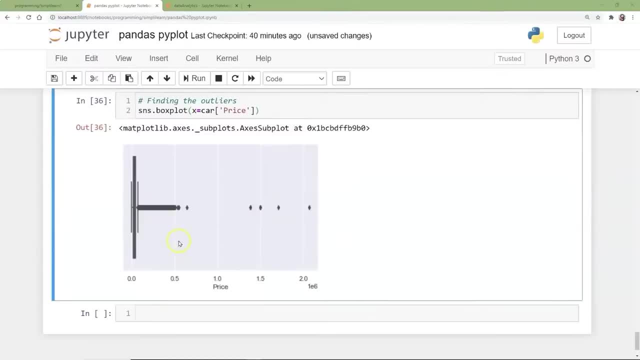 expensive, high end car is what we're looking at. If you were doing fraud analysis, you would be jumping on all over these outliers. Why are these deviation from the standard? What do these people do? And again, this is probably, like I said, a really high end, expensive car out here. 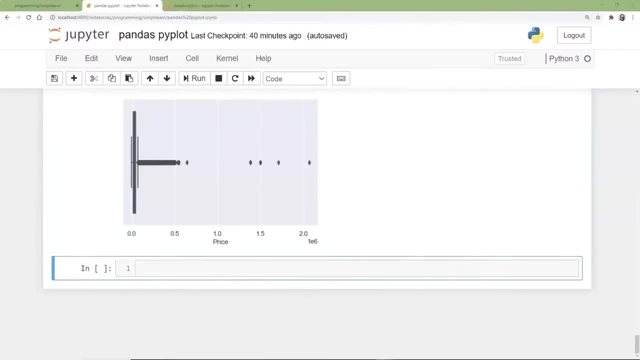 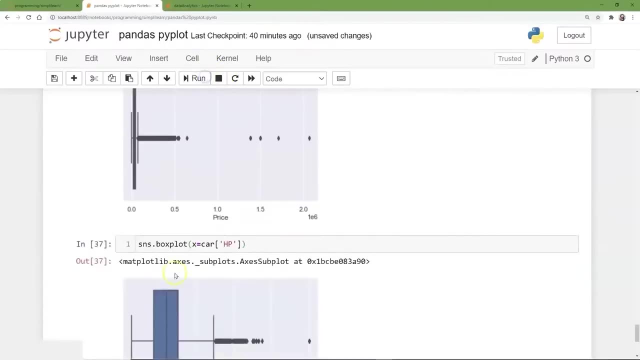 That's what we're looking at And we can also look at the box plot for the horsepower. We'll put that in down here And run that And you can see again: here's our horsepower and it just jumps. And there's these really odd, huge. 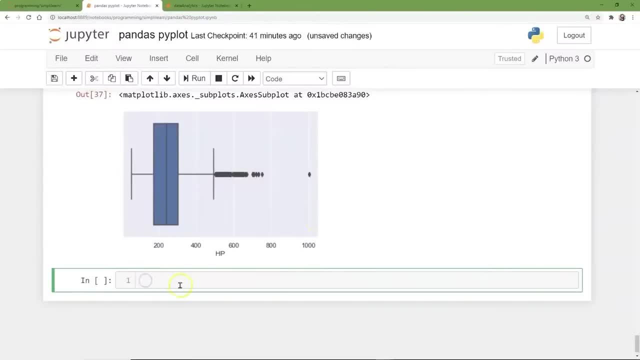 muscle cars out here that are outliers, And we're going to jump into making this a little bit more. as you start displaying your data or your information to your shareholders, We're going to look at plotting a histogram for the number of cars per brand. 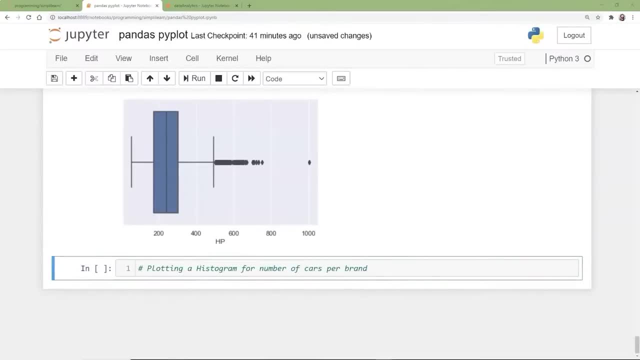 And the first thing we want to go ahead and do is we have with our car. let me go back over here. Here we go. We have our make value counts, largest plot and we want to do a kind equals bar, figure, size, ten, five, And right off the 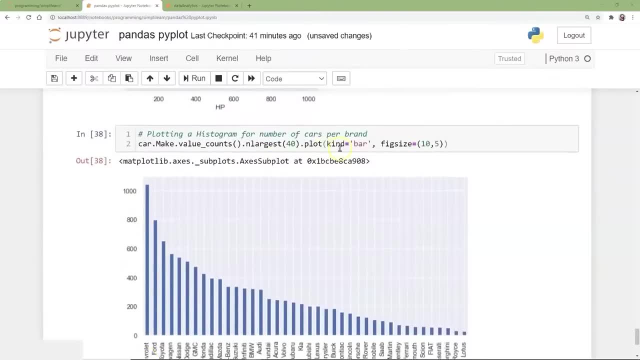 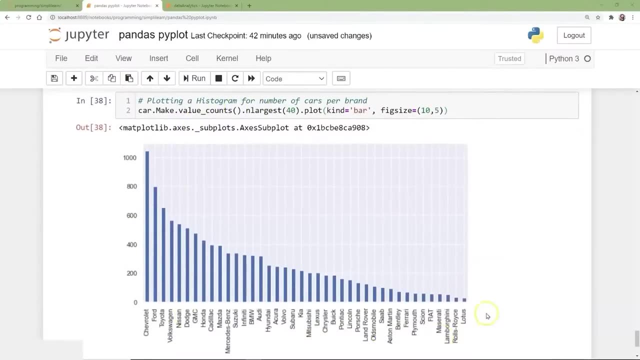 bat. we jump up here and we see Chevrolet is going against what was it? figure race edition. The value counts and we want the largest value. So here's our value counts compared to what the different cars are. Chevrolet puts out a lot of different kinds. 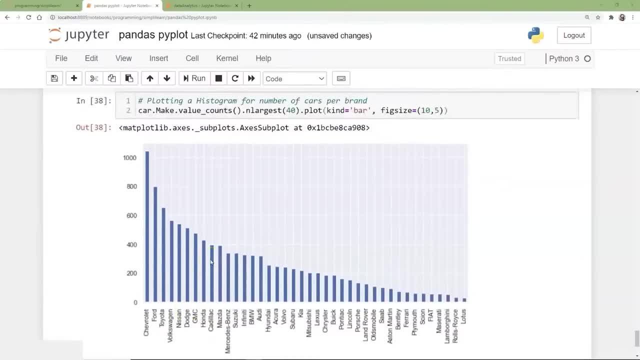 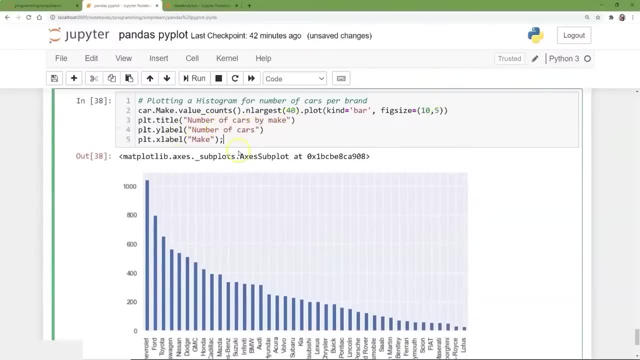 of cars. I didn't realize that they made that many cars Or different types. And then, for readability, let's go ahead and add a title Number of cars by make Number of cars and make. If you had looked at this the first time. 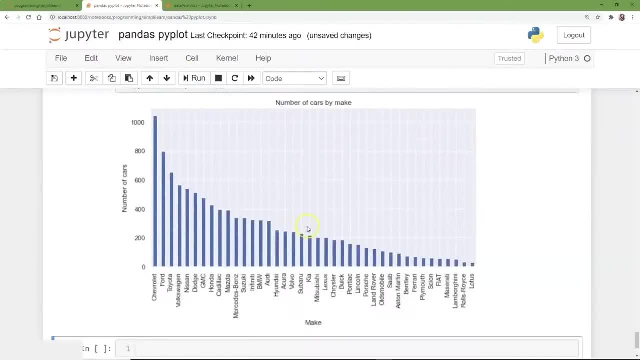 you would have been like: well, what the heck am I looking at? Well, we're looking at the number of cars by make And you can see here now we're talking about the type of cars and the different ones were put out- Lotus, I guess. 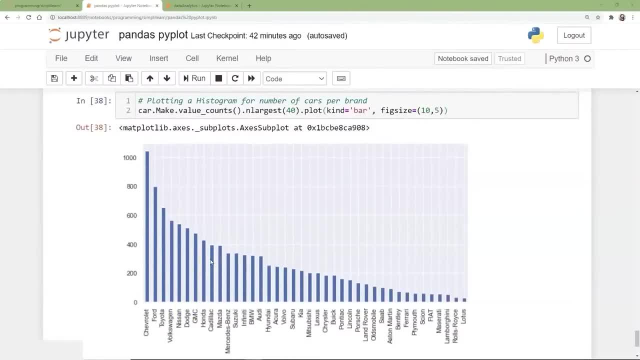 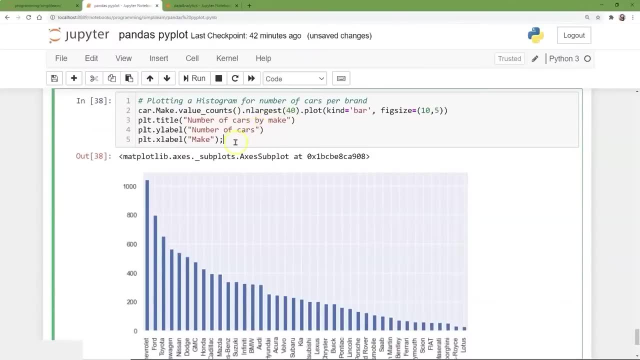 I didn't realize that they made that many cars or different types. and then, for readability, let's go ahead and add a title number of cars by make number of cars and make. if you had looked at this the first time, you would have been like, well, what the heck am I looking at? 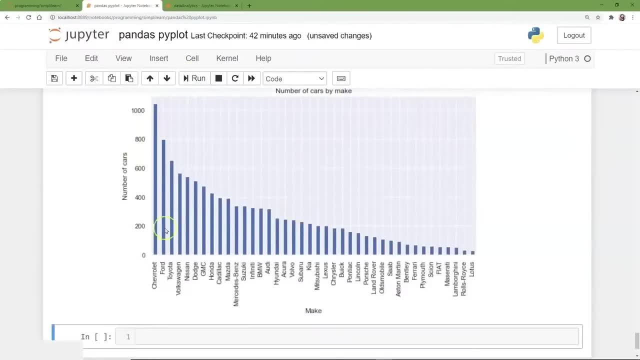 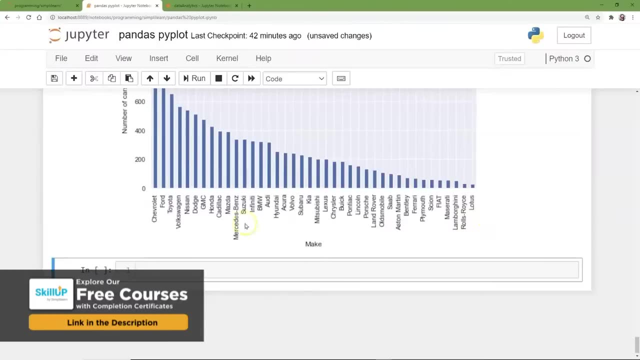 well, we're looking at the number of cars by make and then you can see here. now we're talking about the type of cars and the different ones were put out. Lotus, I guess, only had a few different kinds of cars over there- very high end cars- and then, as doing data analytics, 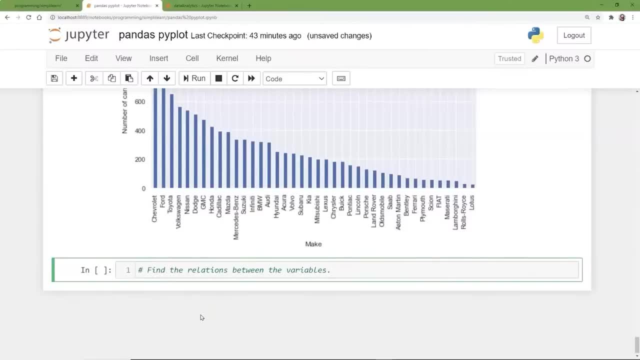 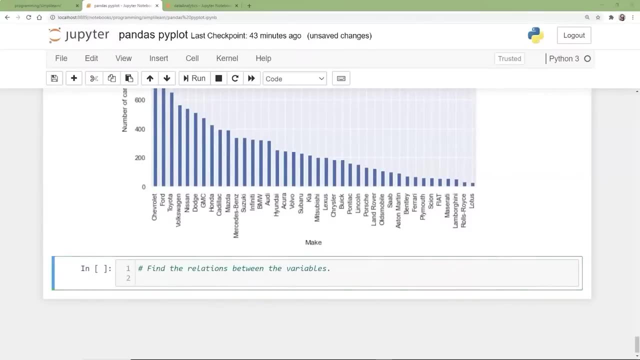 and, as a data scientist, one of the things I am most interested in is the relationship between the variables. so this is always a place to start. we want to know what's going on with our variables and how they connect with each other. so the first thing we're going to do- 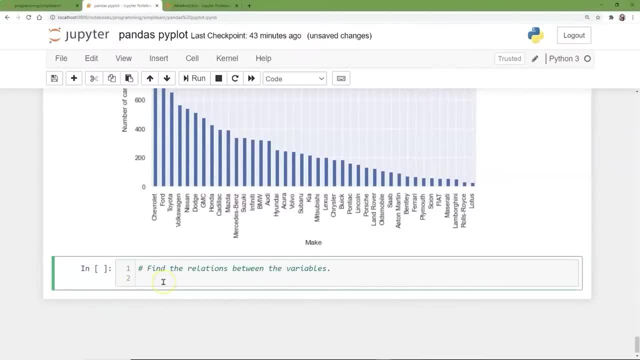 is. we're going to go ahead and set a figure size because we want to make sure it fits our graph. we'll just go ahead and set this one plot figure set to figure size 2010. if you've never used the map plot library, which is sitting behind Seabourn, 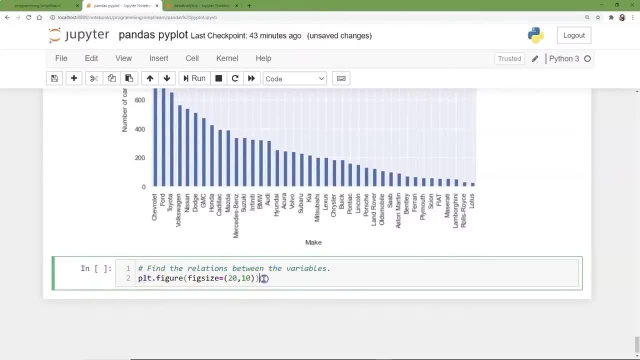 whatever is in the PLT, this is what's loaded. it's like a canvas you're painting on. so the second you load that pie plot as PLT. anything you do to that is affecting everything on it. and then we want to go ahead, since we're using Seabourn. 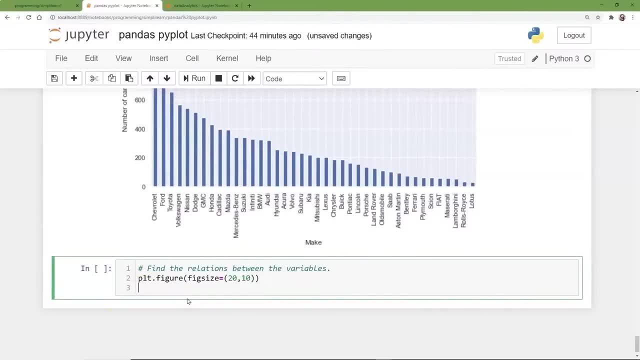 we'll go ahead and create a variable C for relationships or correspondence and carcorr. that's a correlation in Seabourn on top of pandas. again one line and you get the whole correlation on there. and because we're working with Seabourn, let's put it into a nice heat map. 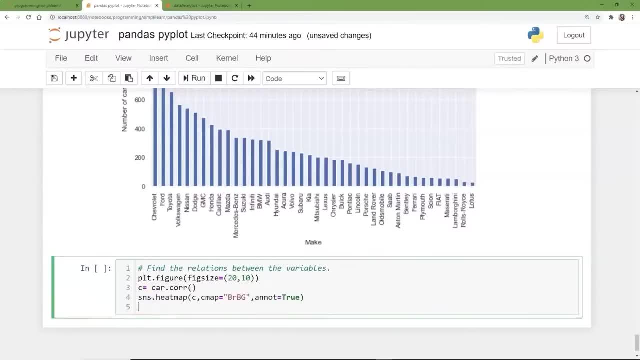 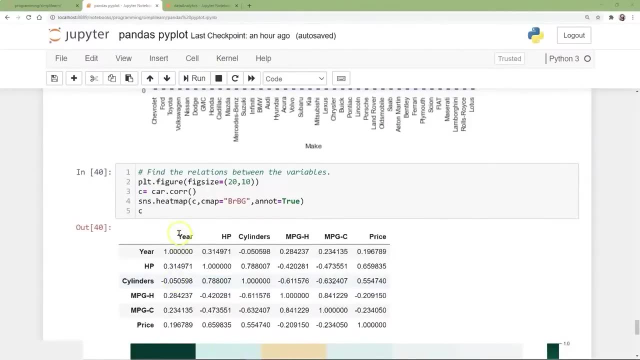 if you're not familiar with heat maps, that means we're just using color as part of our setup. so we have a nice visual and we can see here that the Seabourn, connected to the pandas, prints out a nice chart. we'll talk a little bit about the color here in a second. 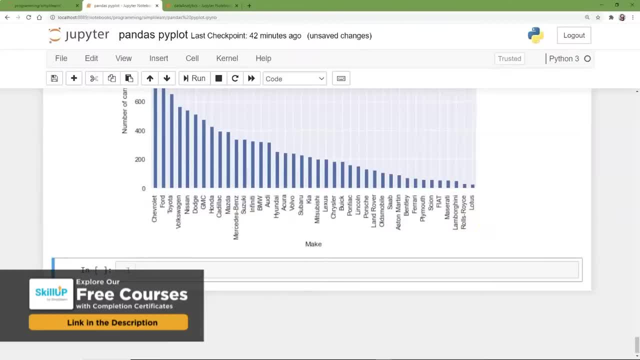 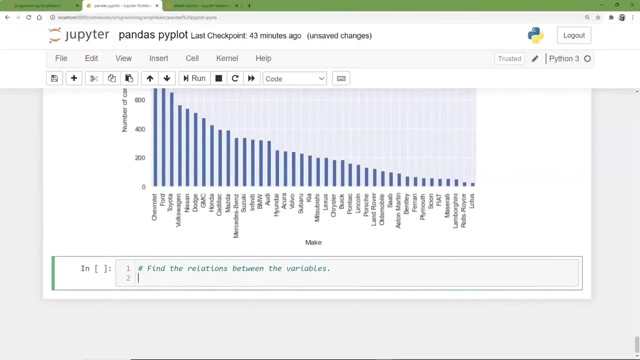 only had a few different kinds of cars over there- Very high end cars- And then, as doing data analytics and as a data scientist, one of the things I am most interested in is the relationship between the variables. So this is always a place to start. We want to know what's. 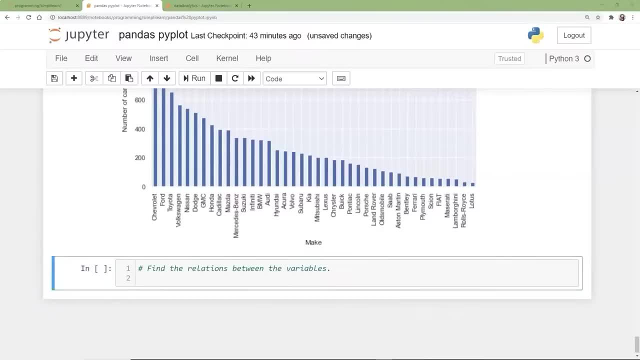 going on with our variables and how they connect with each other. So the first thing we're going to do is we're going to go ahead and set a figure size because we want to make sure it fits our graph. We'll just go ahead and set this one. 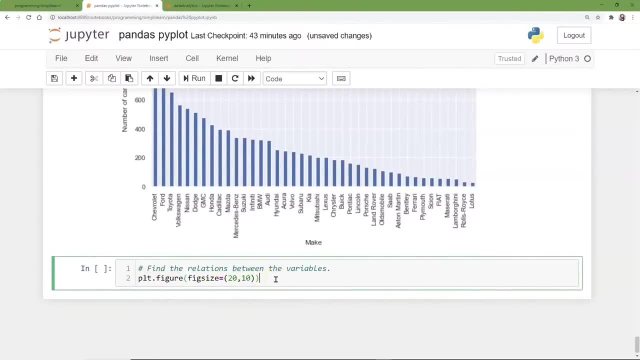 plot figure set to figure size 2010.. If you've never used the map plot library, which is sitting behind Seaborn, whatever is in the PLT, this is what's loaded. It's like a canvas you're painting on. So the second you. 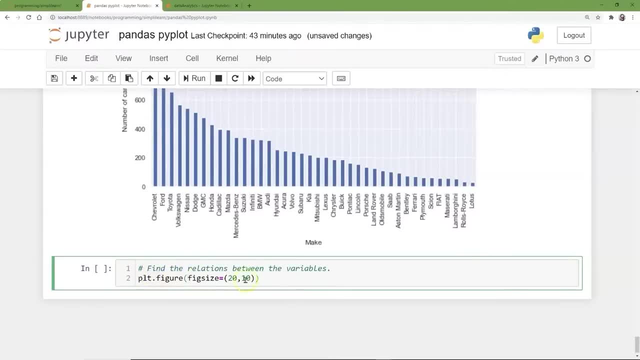 load that pie plot as PLT. anything you do to that is affecting everything on it. And then we want to go ahead. since we're using Seaborn, we'll go ahead and create a variable C for relationships or correspondence And carcorr. that's a correlation in. 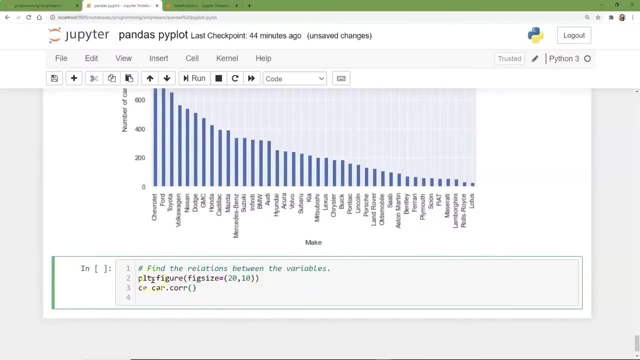 Seaborn on top of pandas. Again one line and you get the whole correlation on there. And because we're working with Seaborn, let's put it into a nice heat map. If you're not familiar with heat maps, that means we're. 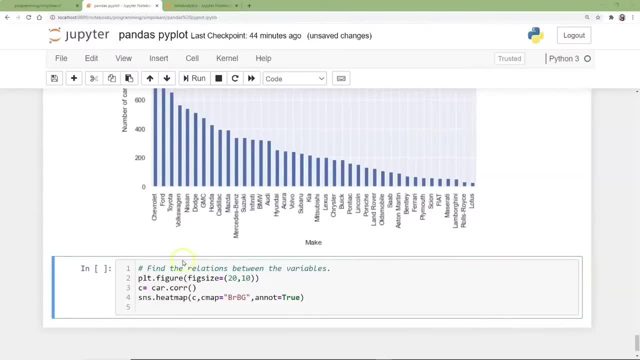 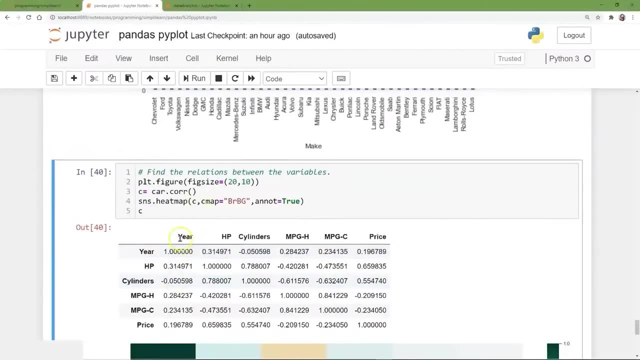 just using color as part of our setup. so we have a nice visual And we can see here that the Seaborn, connected to the pandas, prints out a nice chart. We'll talk a little bit about the color here in a second. It prints out a nice 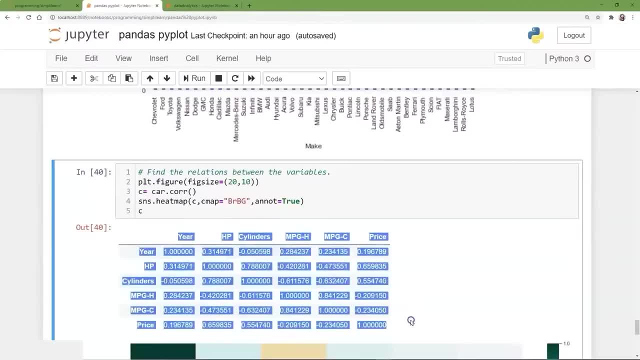 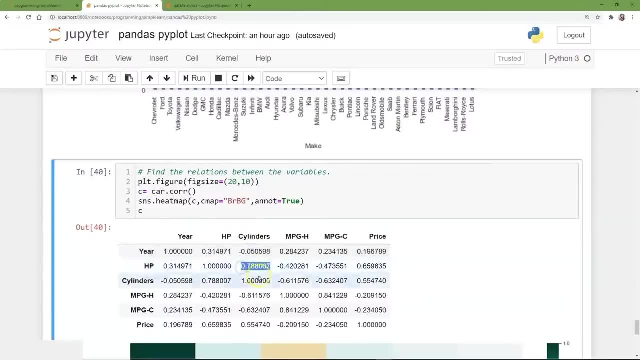 chart. This is the chart I look at As a data scientist. these are the numbers I want to look at And we'll just highlight one of them. Here's cylinders versus horse power. The closer to one, the higher the correlation, So .788. 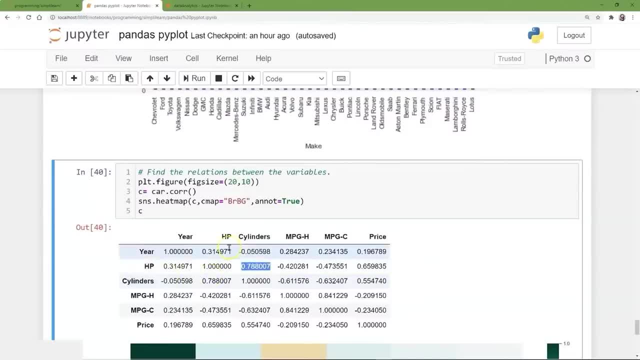 Pretty high correlation between the number of cylinders and how heavy the horse power is. I'm betting, if you looked at the year versus horse power, we can just look at that one Here's year and horse power: .314. not so much, but if you combine them, 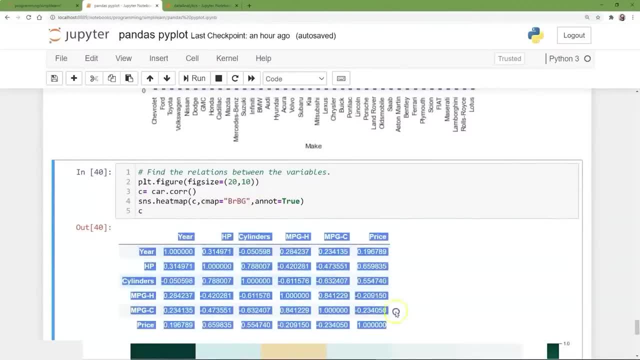 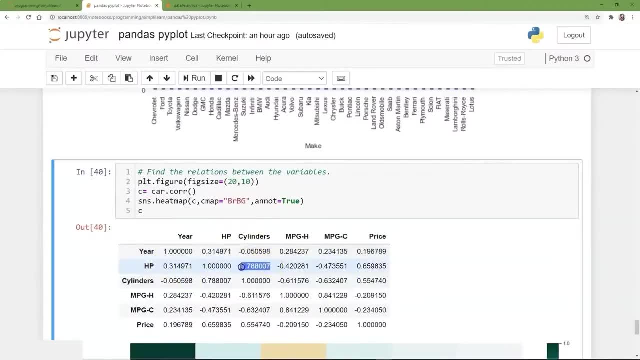 it prints out a nice chart. this is a chart I look at as a data scientist. these are the numbers I want to look at and we'll just highlight one of them. here's cylinders versus horsepower: the closer to one, the higher the correlation, so 0.788. 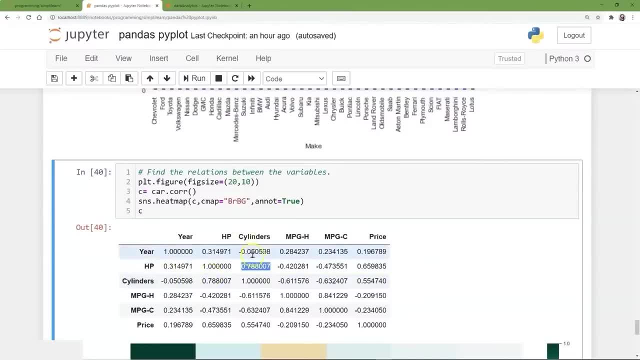 pretty high correlation between the number of cylinders and how heavy the horsepower is. I'm betting, if you looked at the year versus horsepower, we can just look at that one here's year and horsepower: 0.314. not so much, but if you combine them you don't actually add them. 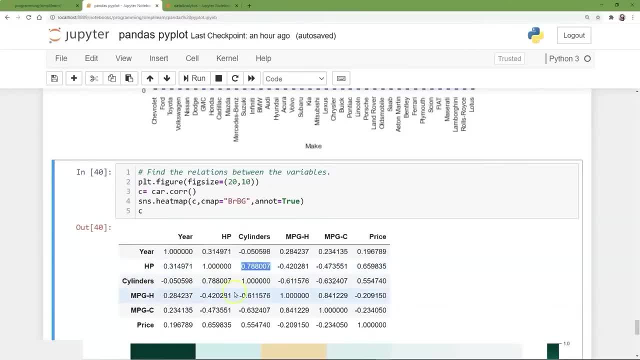 but if you combine them you'll start to see an increase in horsepower per year in cylinders. you could probably get a correlation there and just like 0.78 is a positive correlation you might notice if we look at cylinders. or let's look at horsepower and mileage. 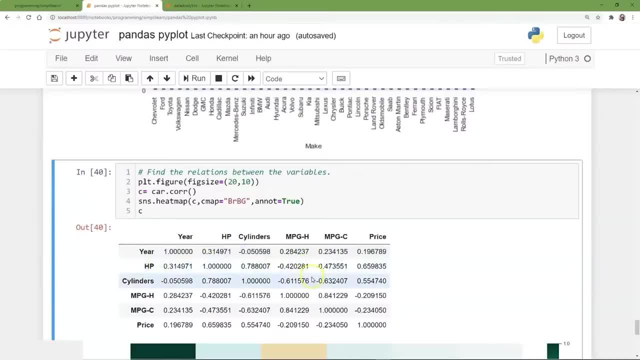 so if we go here to horsepower, to mileage, you get a nice negative. we'll do cylinders, that's a bigger number with cylinders. to the miles per gallon it's a minus 0.6, so it's a negative correlation. the closer to minus one, the more the negative correlation is. 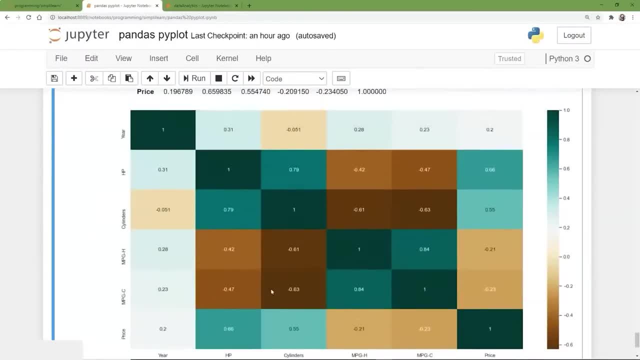 and then the chart you would actually show people is a nice heat map. this is all our colors and it's just those numbers put into a heat map. the darker the color, the higher the correlation. you can see straight down the middle. obviously the year correlates directly with the year. 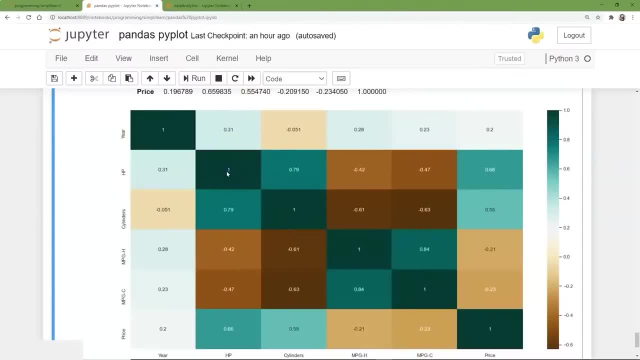 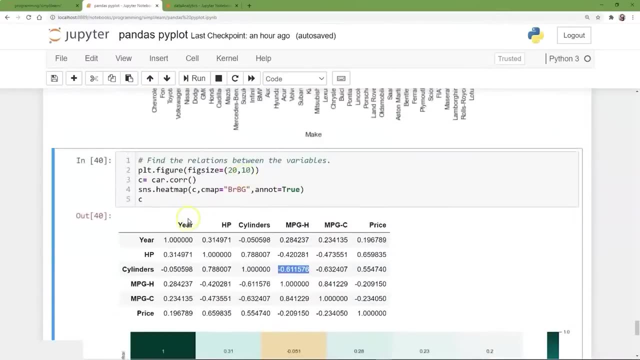 horsepower with horsepower and so on. that's why it's a one. the closer to the one, the higher the correlation between the two pieces of data. now, this is a good example, a good introduction. pandas goes way beyond this, most of the functionality in numpy, since panda sits on it. 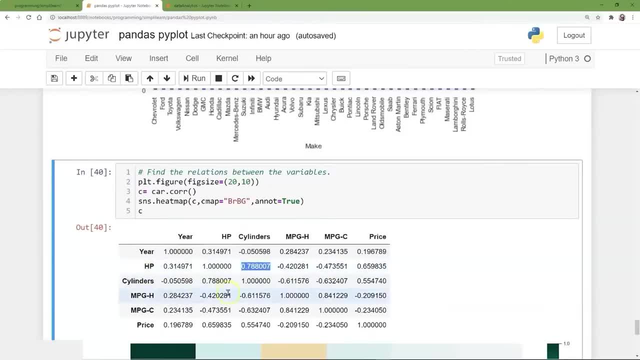 you don't actually add them, But if you combine them you'll start to see an increase in horse power per year in cylinders. You could probably get a correlation there And just like .788 is a positive correlation you might notice if we look at cylinders. 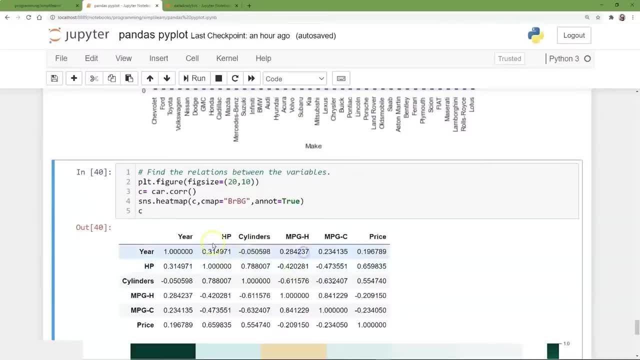 or let's look at horse power and mileage. So if we go here to horse power, to mileage, you get a nice negative. we'll do cylinders, that's a bigger number with cylinders to the miles per gallon it's a minus .6.. So it's a negative. 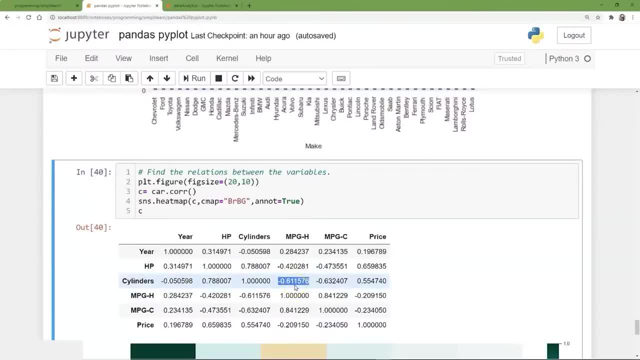 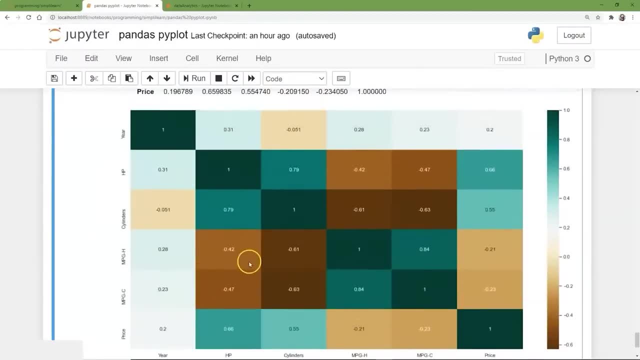 correlation. The closer to minus one, the more the negative correlation is. And then the chart you would actually show people is a nice heat map. This is all our colors and it's just those numbers put into a heat map. The darker the color, the higher the correlation. 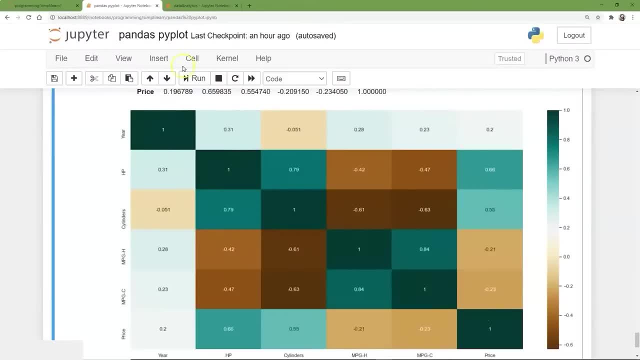 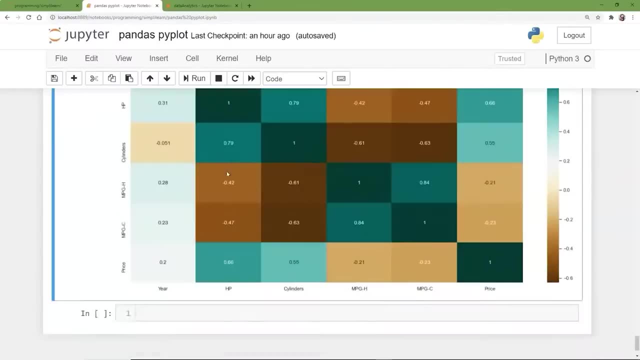 You can see straight down the middle. obviously, the year correlates directly with the year, horse power with horse power, and so on. That's why it's a one. The closer to the one, the higher the correlation between the two pieces of data. Now this is: 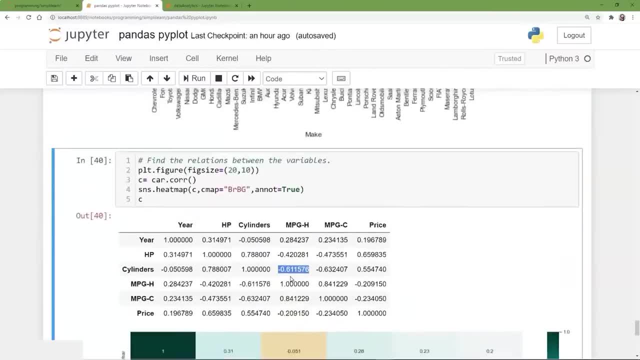 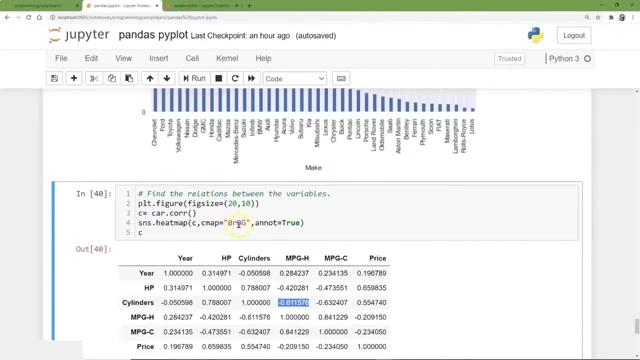 a good introduction. Pandas goes way beyond this. Most of the functionality in NumPy, since Pandas sits on, it, is also in Pandas, and then it even has additional features in it And we use Seaborn pretty extensively, sitting on top over our 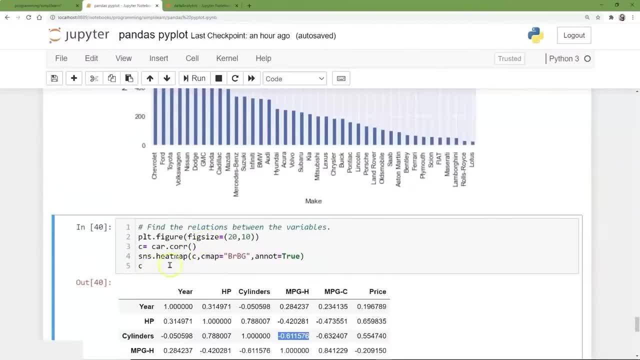 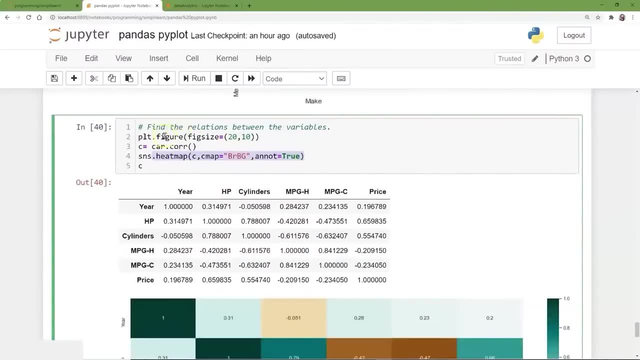 is also in pandas, and then it even has additional features in it and we use seaborn pretty extensively, sitting on top over our pi plot. so keep in mind that our pi plot has a ton of other features in it that we didn't even touch on in here. 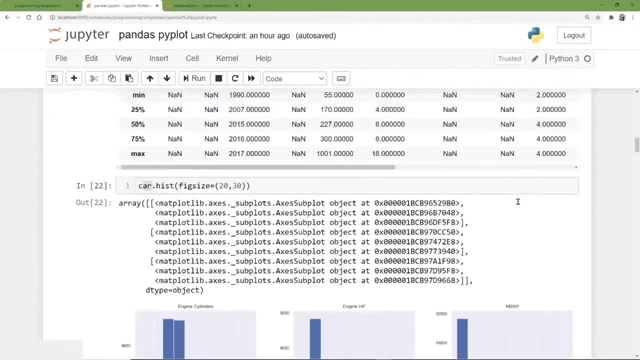 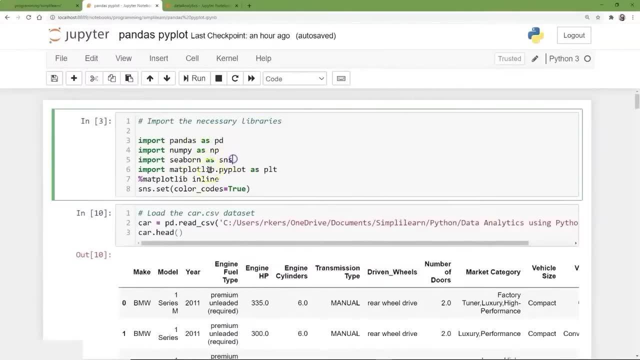 we couldn't, even if you had a sole course in it. there's just so many things hidden in there, depending on what your domain you're working on. but you can see here here's our seaborn and here's our matplot library. that's all our graphics, that we did. 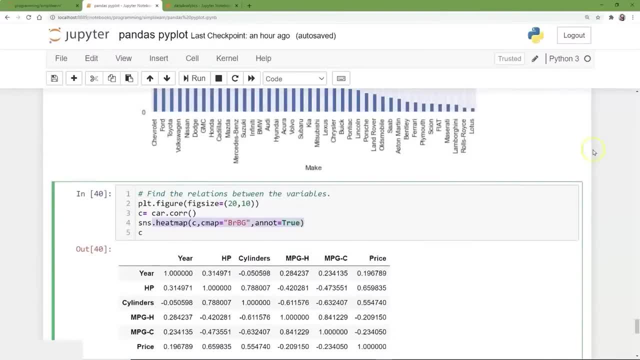 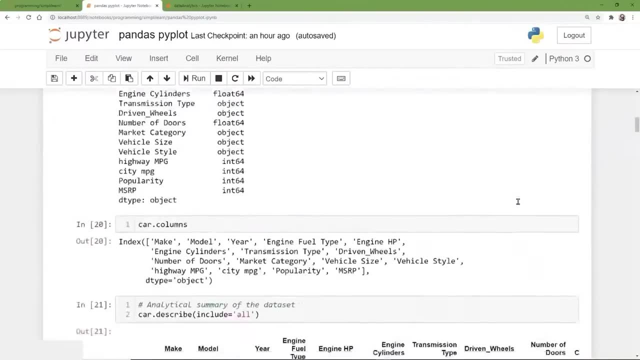 Pi plot. So keep in mind that our Pi plot has a ton of other features in it that we didn't even touch on in here. We couldn't, even if you had a sole course in it. there's just so many things hidden in there, depending on what your domain you're. 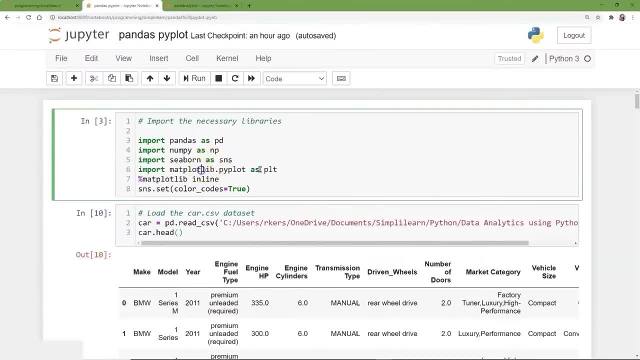 working on. But you can see here, here's our Seaborn and here's our Matplot library. That's all our graphics, that we did. And then the Seaborn works really nicely with the Pandas. We really like that. So that wraps up our demo. 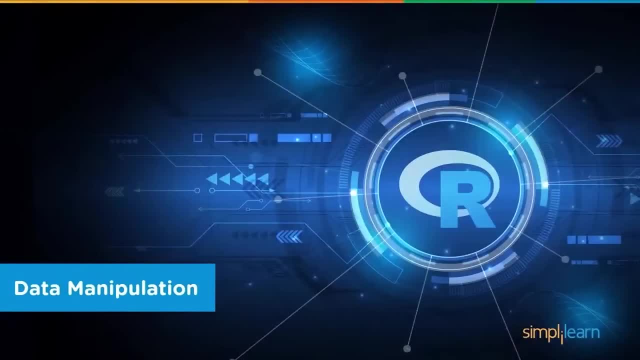 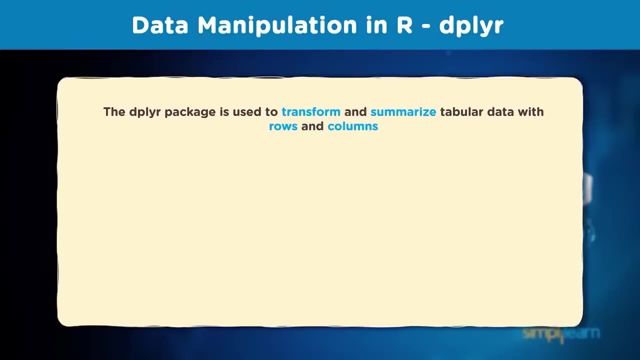 part for today. Let's learn about data manipulation in R, and here we will learn about dplyr package. And when we talk about this dplyr package, it is much faster and much easier to read than base R, So dplyr package is used. 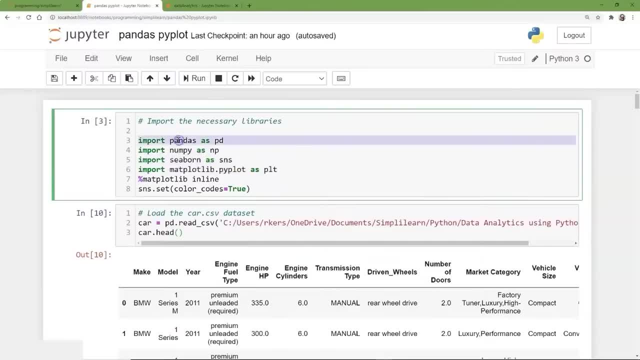 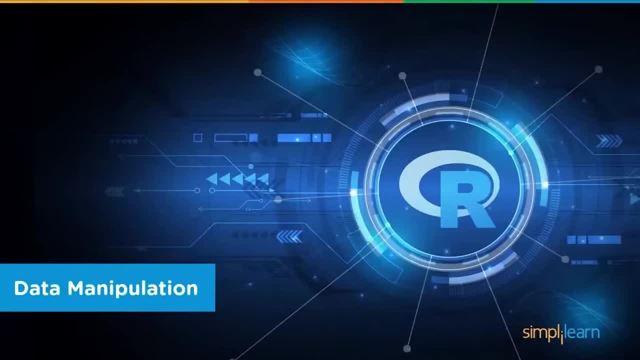 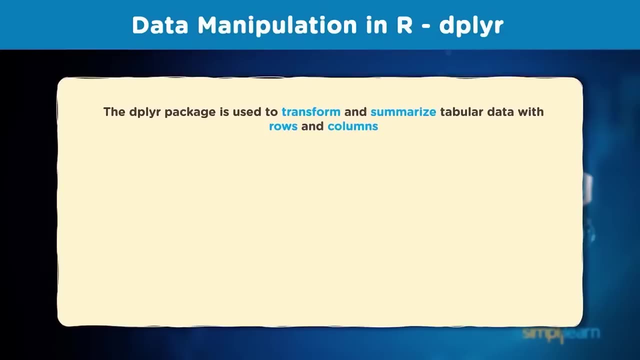 and then the seaborn works really nicely with the pandas. we really like that. so that wraps up our demo part for today. let's learn about data manipulation in R, and here we will learn about dplyr package and when we talk about this dplyr package. 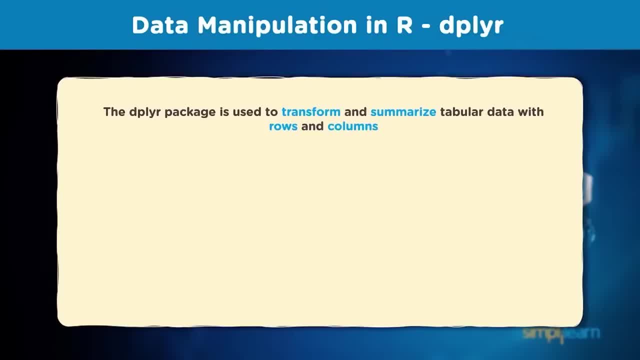 it is much faster and much easier to read than base R. so dplyr package is a. so dplyr package is used to transform and summarize tabular data with rows and columns. you might be working on a data frame or you might be getting in a inbuilt R data set. 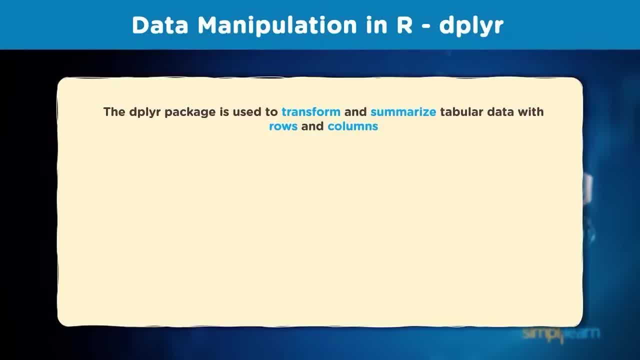 which can then be converted into a data frame. so we can get this package dplyr by just calling in library function and this can be used for grouping by data, summarizing the data, adding new variables, selecting different set of columns, filtering our data sets, sorting it. 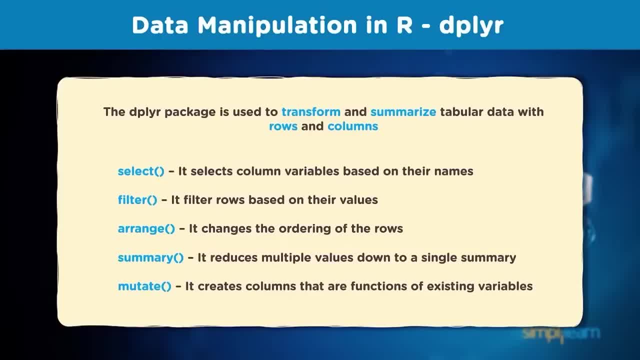 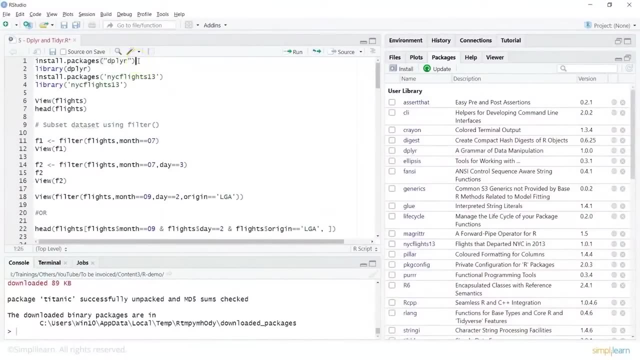 selecting it, arranging it or even mutating. that is basically creating new columns using functions on existing variables. so let's see how we work with dplyr now. here I can basically get the package here. so I can just say: install dot packages, dplyr. now we already see the package here. 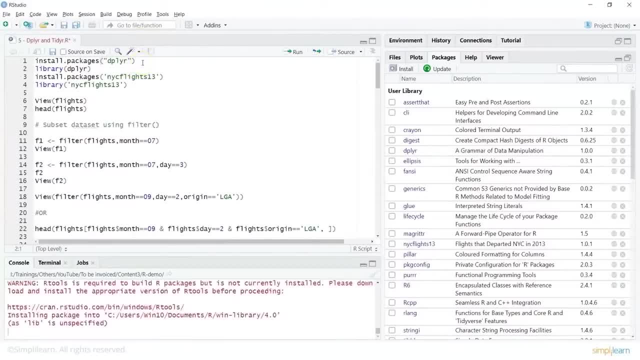 which is showing up, so I will just select this one. I can do a control enter and that will basically set up the package. package dplyr successfully unpacked. so that is done. now you can start using this package by just doing a library dplyr. 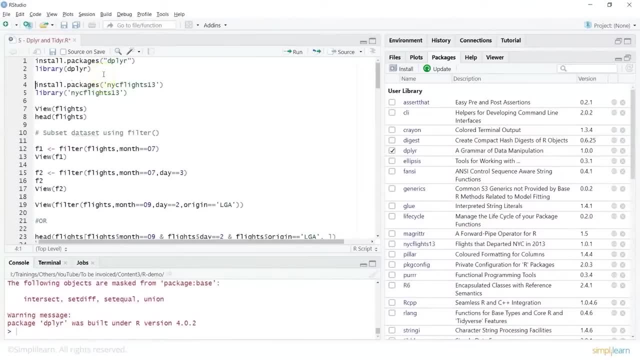 and this was built. it shows me my version of R. so let's also use a inbuilt data set that is New York flights 13. so we can do install dot packages and that will search and get that relevant data set. I can again call it by using library function. 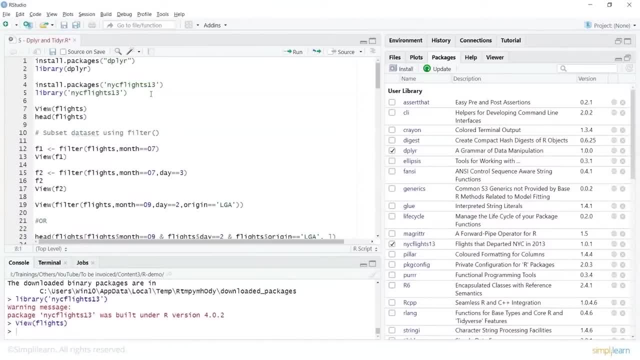 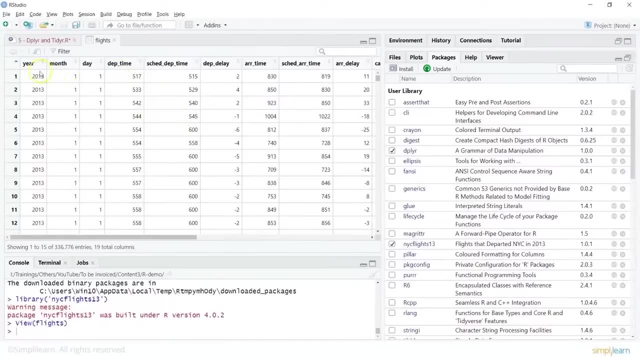 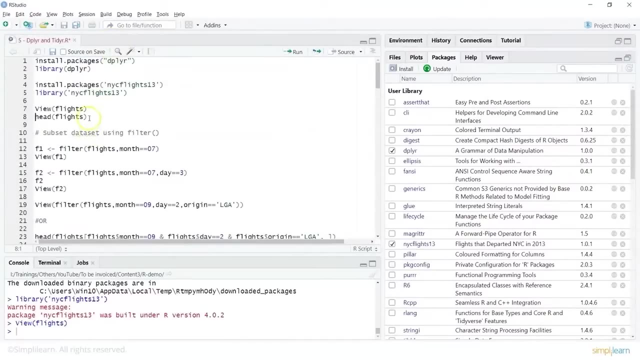 now, once that is done, we can look at some sample data here by just doing view flights and that shows me the data in a neat and a tabular format which shows me year, month, day, departure time, scheduled departure time and so on. now we can also do a head. 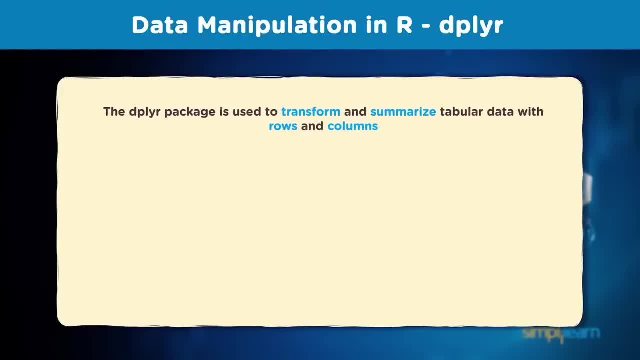 to transform and summarize tabular data with rows and columns. You might be working on a data frame or you might be getting in a inbuilt R data set which can then be converted into a data frame. So we can get this package dplyr by just. 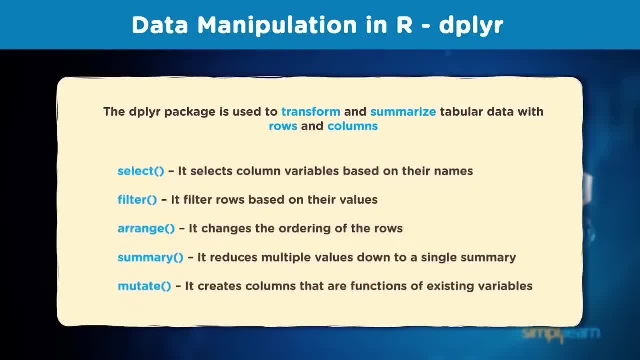 calling in library function, And this can be used for grouping by data, summarizing the data, adding new variables, selecting different set of columns, filtering our data set, sorting it, selecting it, arranging it or even mutating. That is basically creating new columns. 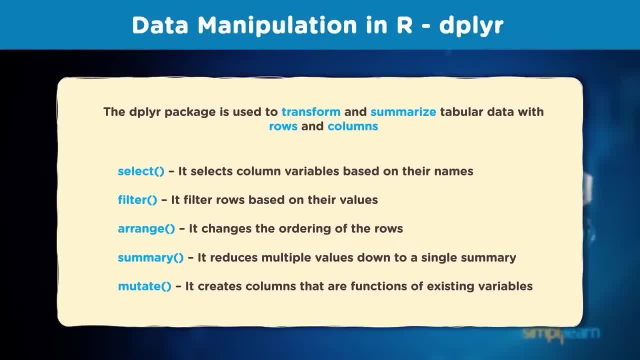 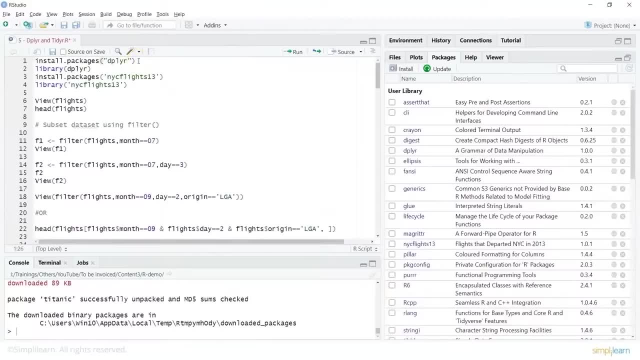 using functions on existing variables. So let's see how we work with dplyr. Now here I can basically get the package here. So I can just say: install dot packages, dplyr. Now we already see the package here which is showing up. 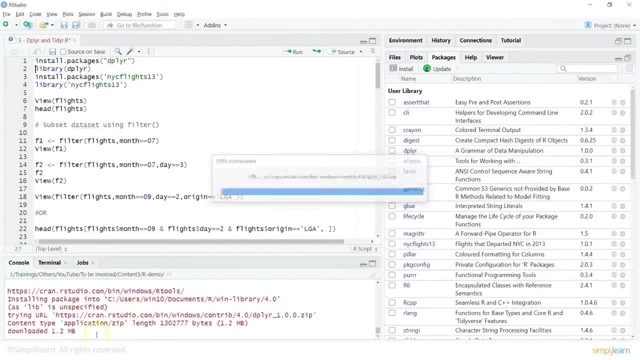 So I will just select this one. I can do a control enter and that will basically set up the package. Package dplyr successfully unpacked. So that is done. Now you can start using this package by just doing a library dplyr. 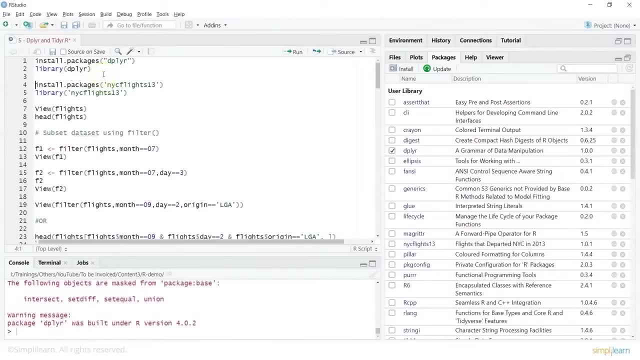 and this was built. It shows me my version of R, So let's also use a inbuilt data set, that is New York flights 13.. So we can do install dot packages and that will search and get that relevant data set. I can again call it by using: 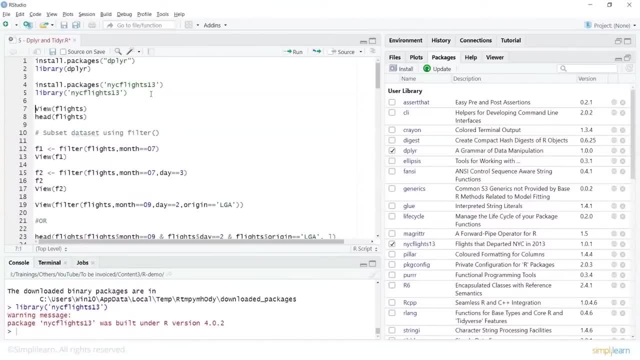 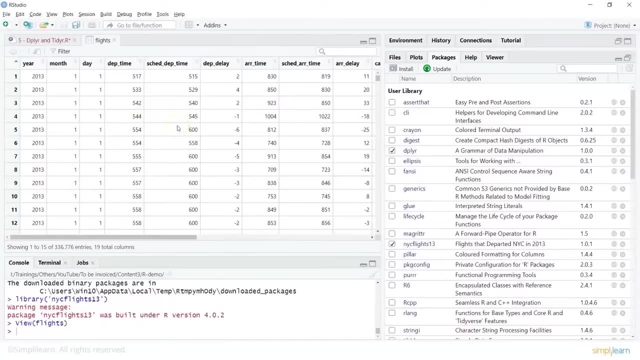 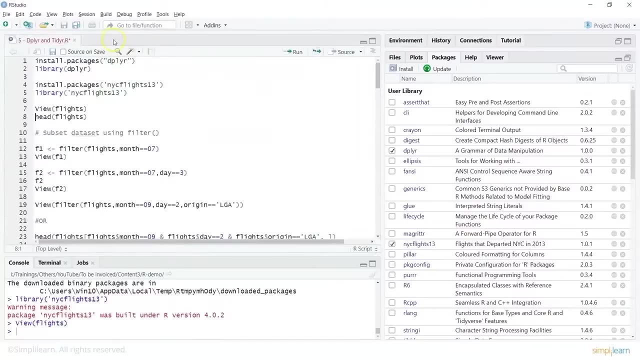 library function. Now, once that is done, we can look at some sample data here by just doing view flights and that shows me the data in a neat and a tabular format which shows me year, month, day, departure time, scheduled departure time and so on. 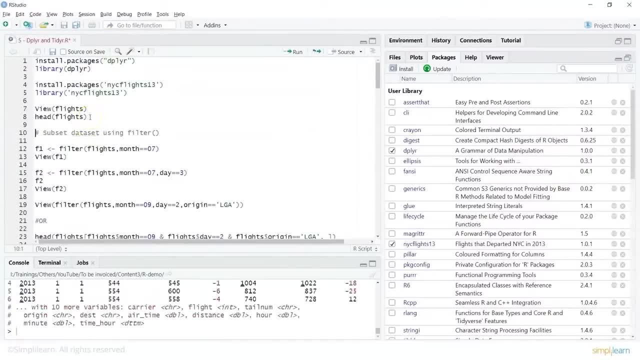 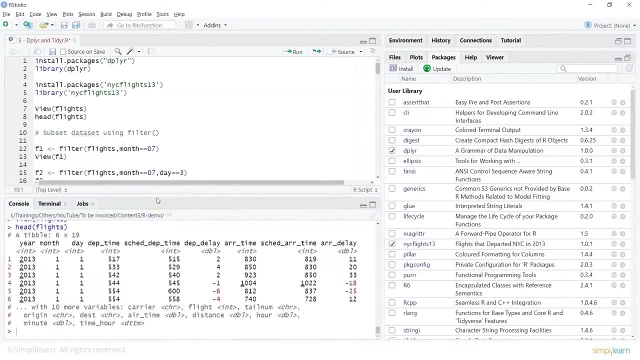 Now we can also do a head to look at some initial data which can help us in understanding the data better. So what is this data about? How many columns we have, What are the data types or object types here? It shows me how many variables. 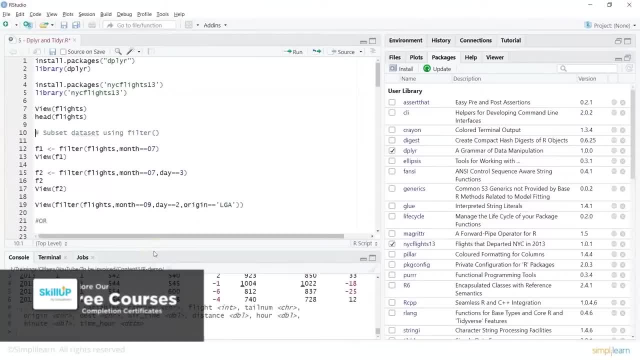 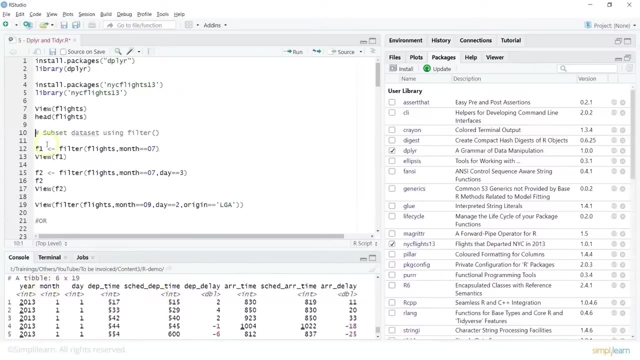 we have. So this is fine. Now we can start using dplyr and in that we can use, say, filter function if we would want to look in for specific value. Now here we have the column as month, so I will do a filter Now I am creating 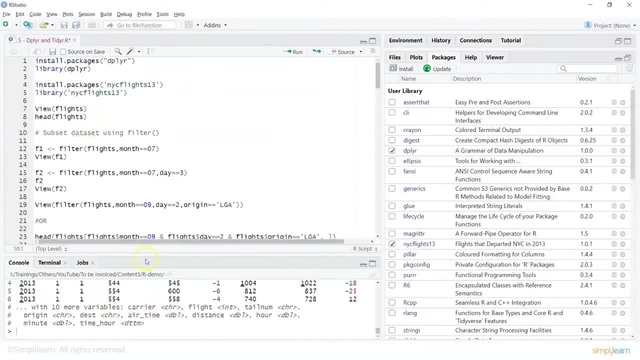 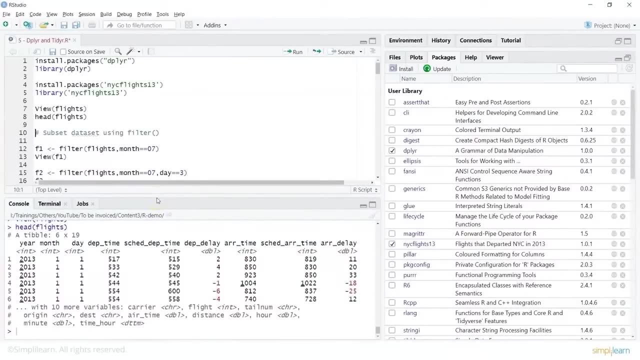 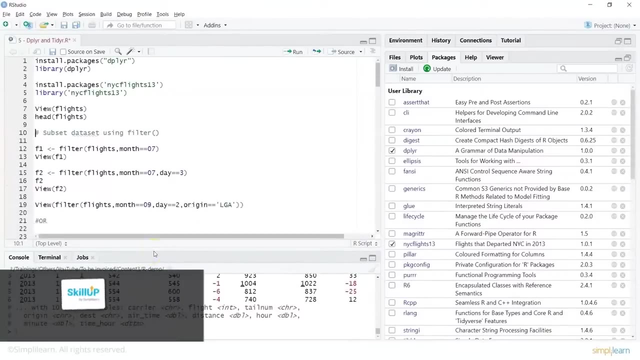 to look at some initial data which can help us in understanding the data better. so what is this data about? how many columns we have, what are the data types or object types here? it shows me how many variables we have. so this is fine. now we can start using dplyr. 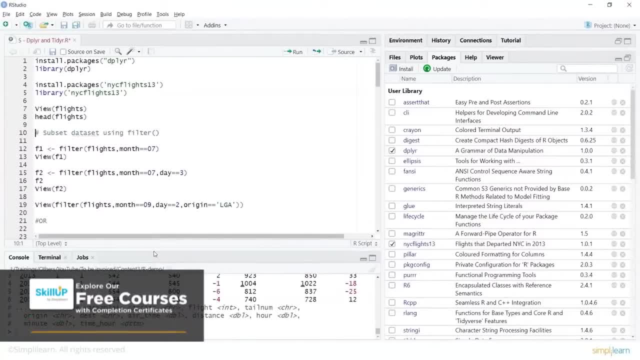 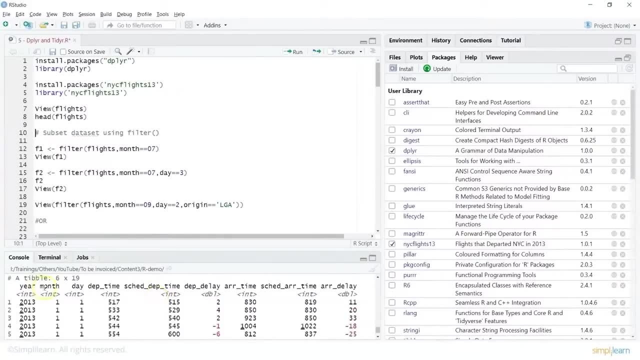 and in that we can use, say, filter function if we would want to look in for specific value. now here we have the column as month, so I will do a filter. now I am creating a variable f1. I am using the filter function on flights, which we already have. 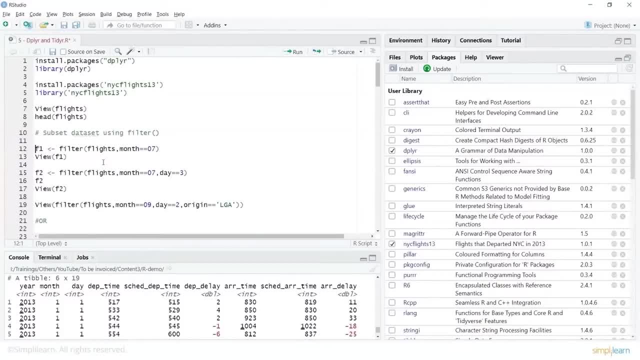 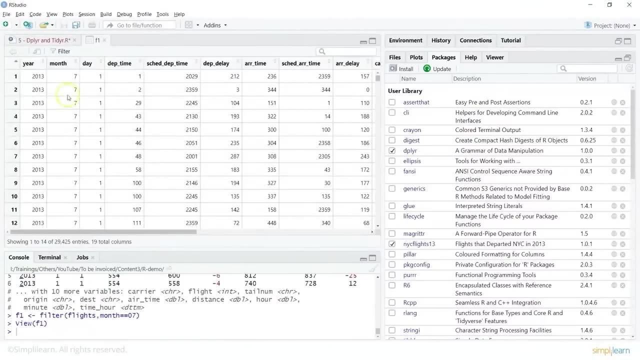 and then what we can do is we can basically look at the month where the month value is 07. so let's look at that and this one. you can do a view on f1, which shows me the data wherein you have filtered out all the data based on month being 7. 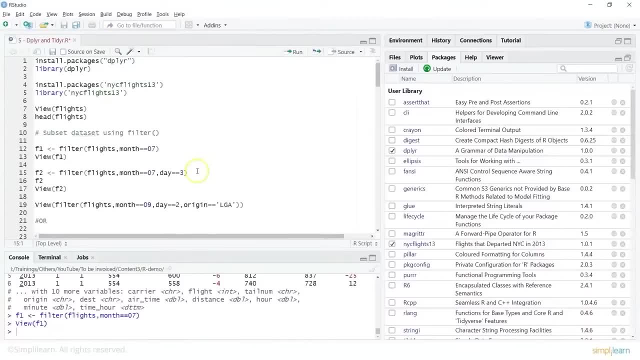 so this is a simple usage of filter. we can take some other example. we may want to introduce and include multiple columns so we can say f2 filter flights and here we will say month is equal to 7, day is 3, and then look at the value of f2. 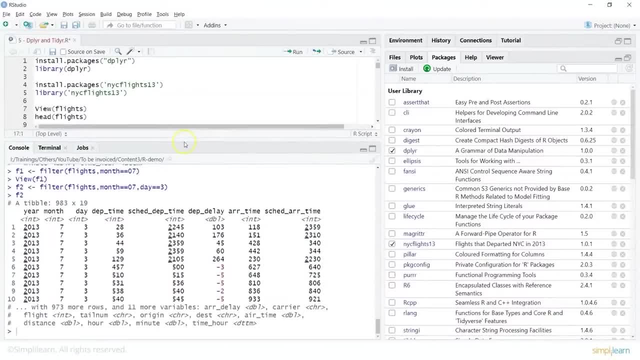 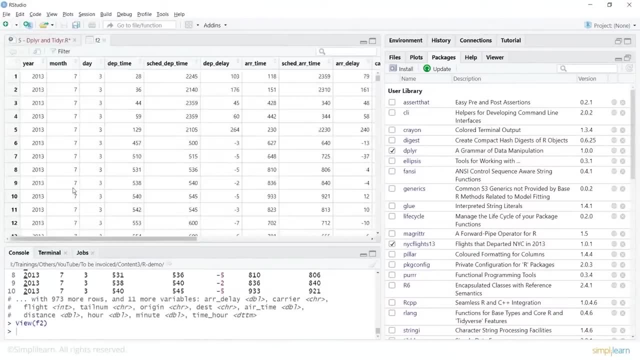 if you are interested in seeing this and that tells you the month is 7 and day is 3. you could also look into a more readable format by using view on f2, and that gives me my selected result. so we are just extracting in some specific value. 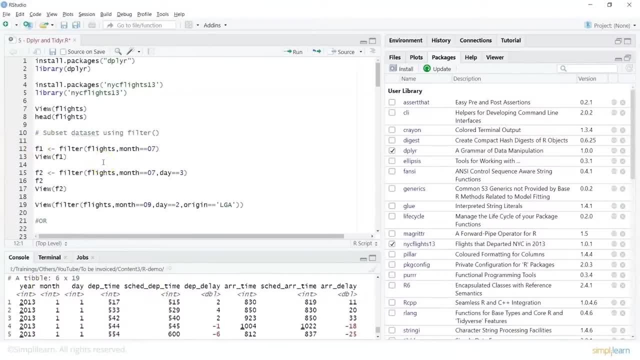 a variable f1.. I am using the filter function on flights, which we already have, And then what we can do is we can basically look at the month where the month value is 07.. So let's look at that and this one. you can do a view. 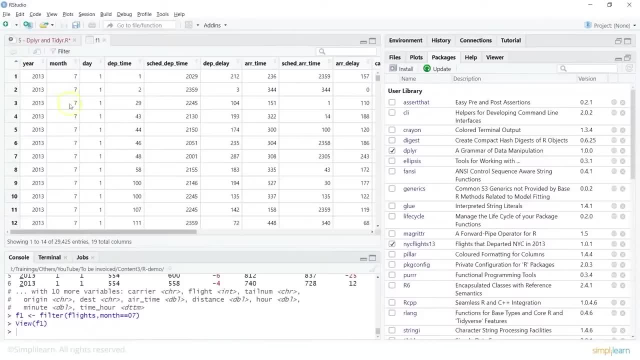 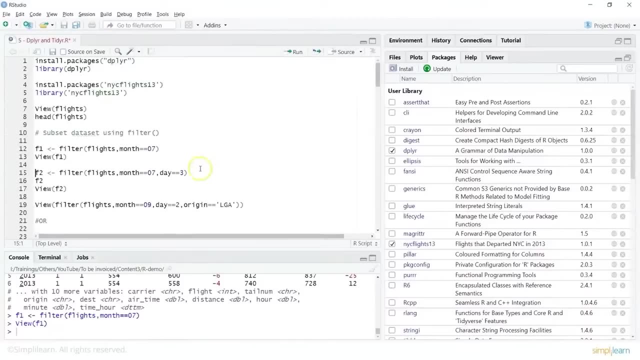 on f1, which shows me the data wherein you have filtered out all the data based on month being 7.. So this is a simple usage of filter. We can take some other example. We may want to include multiple columns, So we can say f2. 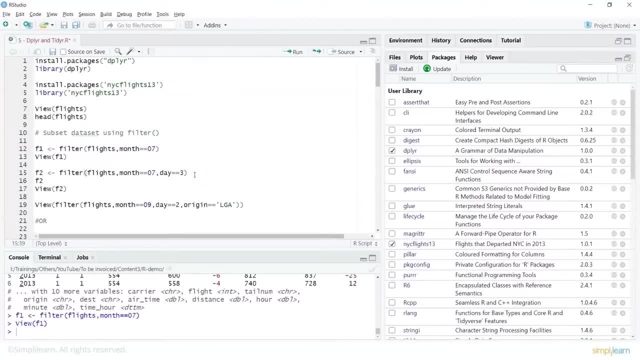 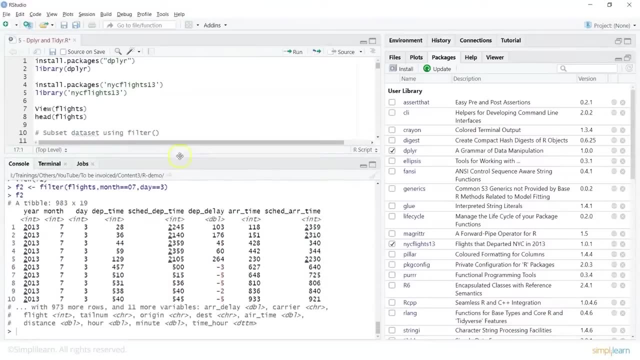 filter flights, and here we will say month is equal to 7, day is 3, and then look at the value of f2, if you are interested in seeing this, and that tells you the month is 7 and day is 3.. You could also 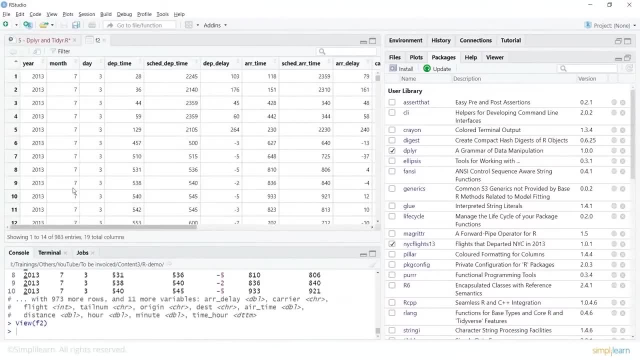 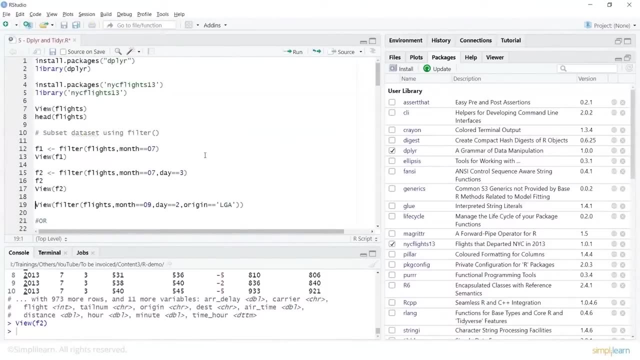 look into a more readable format by using view on f2, and that gives me my selected result. So we are just extracting in some specific value. We can keep extending this, so here we can say: flights is what we would want to work on. I am using the filter function. 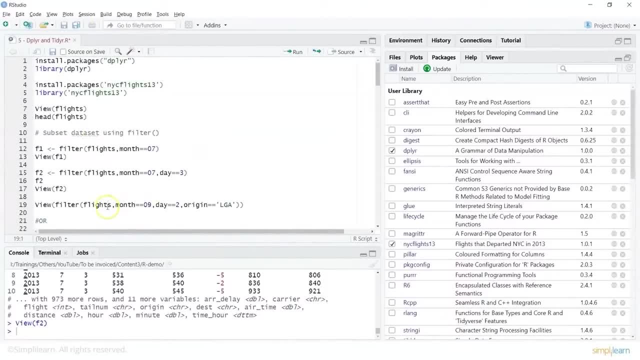 we can keep extending this, so here we can say: flights is what we would want to work on. I am using the filter function so I can straight away, instead of creating a variable, then doing a view, I can also do a view. in this way, I can just pass in my filter. 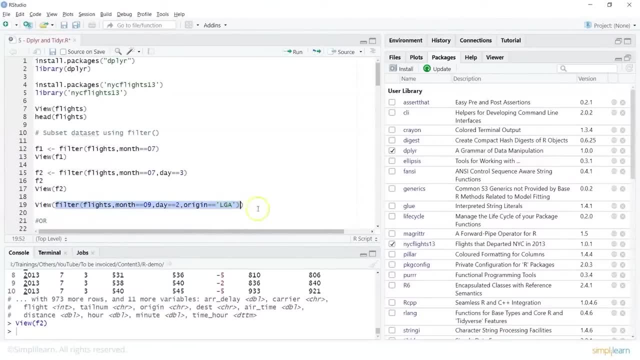 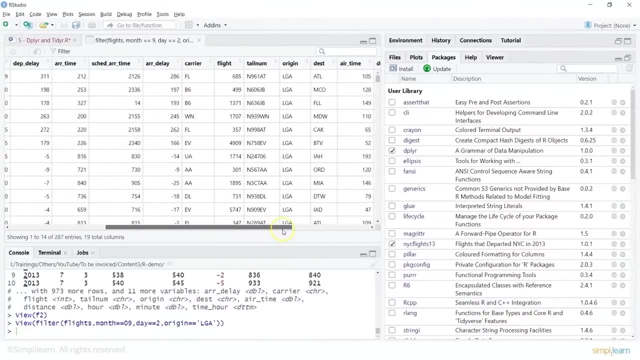 within the view and within this I am saying filter, I would want to look at the flights, month being 09, day being 2 and origin being lga, and then that shows me the value here and obviously you can scroll and look at all the columns and if you see, 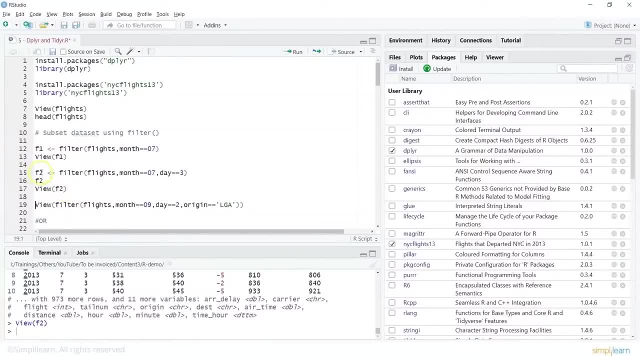 so I can straight away, instead of creating a variable, then doing a view, I can also do a view. in this way, I can just pass in my filter within the view, and within this I am saying filter. I would want to look at the flights month being. 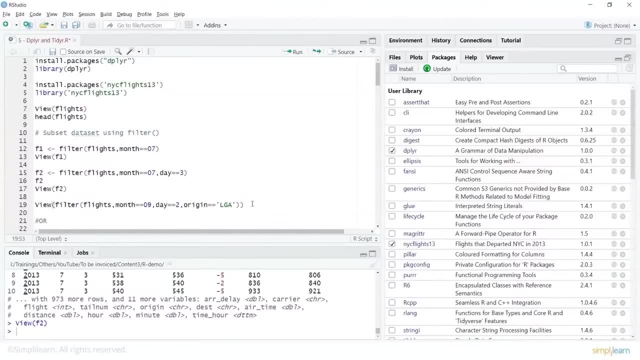 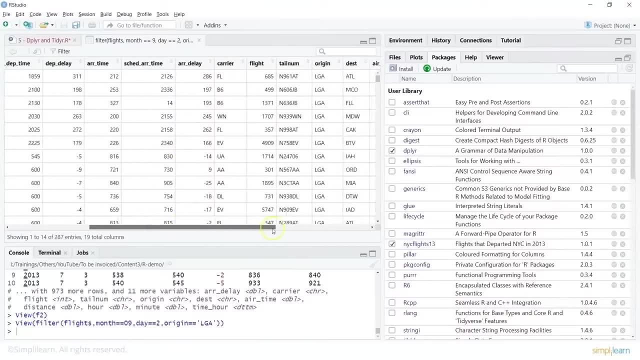 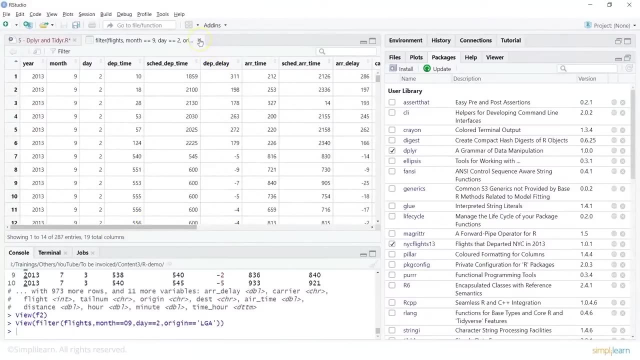 09,, day being 2 and origin being lga, and then that shows me the value here and obviously you can scroll and look at all the columns and if you see the origin column it shows the selected values. So now we have filtered our data. 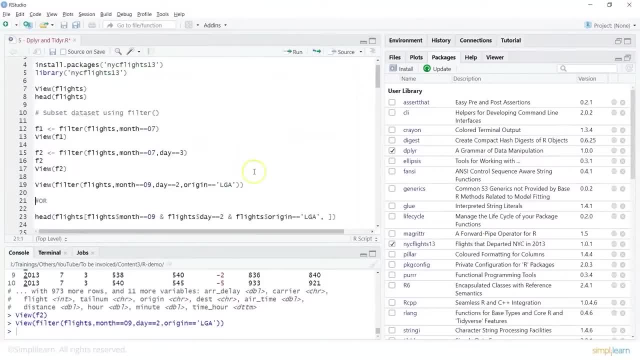 based on values in three different columns. Now what we can also do is we can use AND or. we can use OR operators, So I could have done this in a little different way. So I could have said head, which shows me initial result. I will do a flights. 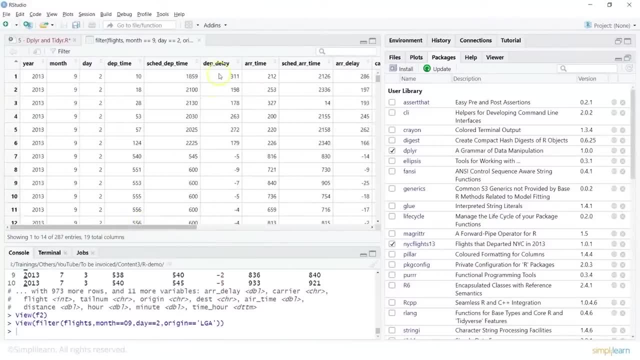 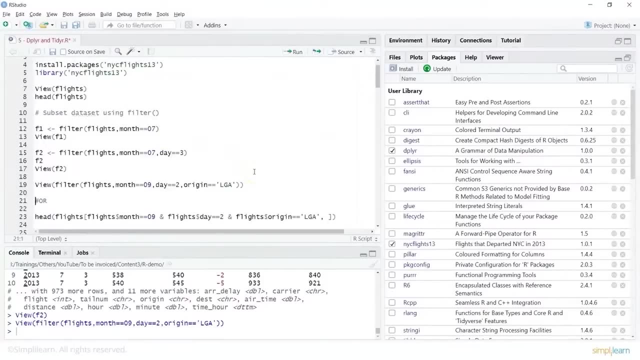 the origin column, it shows the selected value. so now we have filtered our data based on values in 3 different columns. now what we can also do is we can use and, or we can use or operators, so I could have done this in a a little different way. 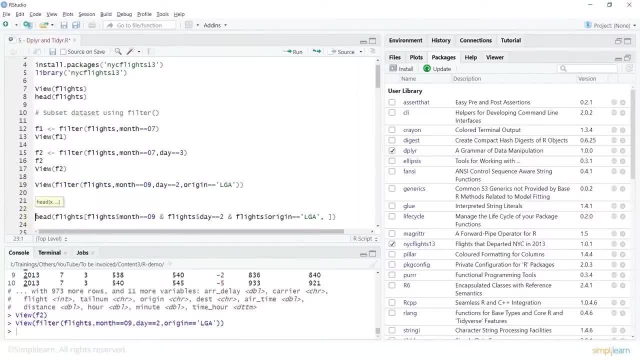 so I could have said here, so I could have said head, which shows me initial result, I will do a flights. so within my head function I am passing in this. and what does that contain? so you are saying flights and in this flights data set you would want to pick up the month. 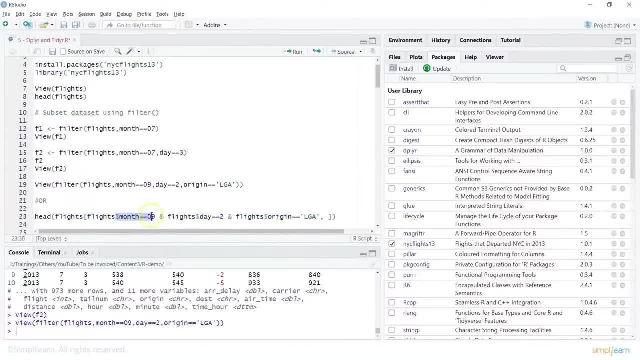 being the column. so we use the dollar symbol here. we give in a value and I will say and, and I will again say flights, wherein I will select the day being 2, and, and, and remember when you talk about, and. it is going to check if all the values are met, true. 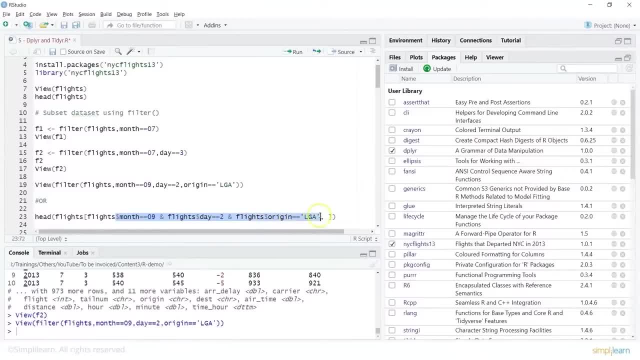 so then you say flights origin lgea and you look at the value. so in this way I can filter out specifically multiple values by specifying columns. now, we could have done it in this way, we could have created a view or we could have assigned this to a variable. 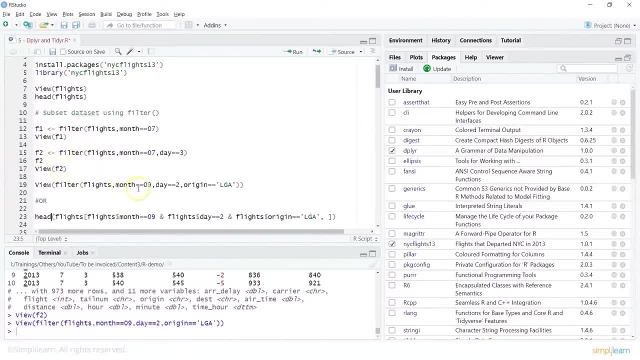 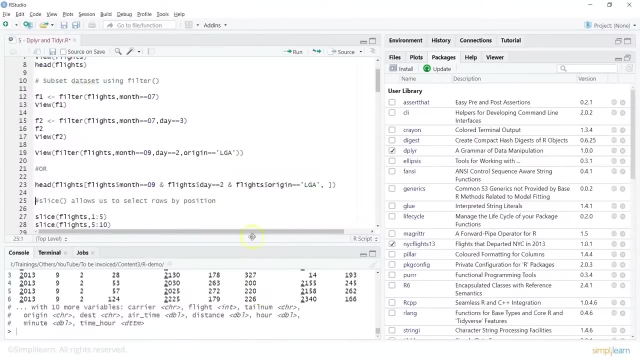 and then done a view on that, where we could have selected month being day and origin, or you can be more specific in specifying all the columns. it makes the code more readable. so let's look at the values and here you are looking at head, which shows me based on month. 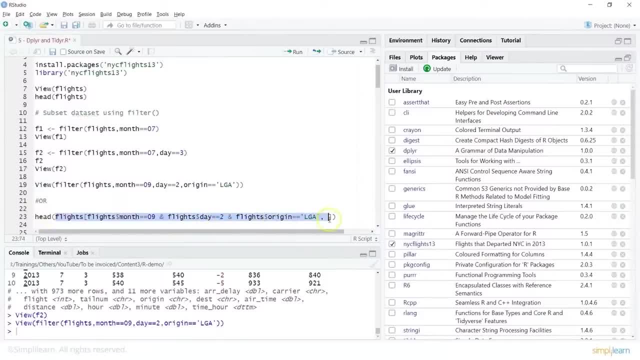 so within my head function, I am passing in this, and what does that contain? So you are saying flights and in this flights data set you would want to pick up the month being the column. So we use the dollar symbol here, We give in a value. 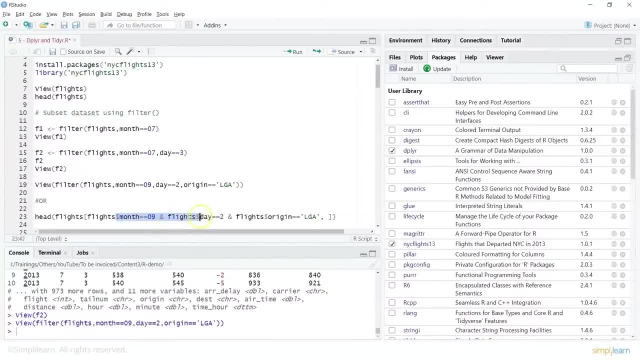 and I will say AND, and I will again say flights, wherein I will select the day being 2 and AND. and remember, when you talk about AND, it is going to check if all the values are met, true. So then you say flights- origin lga and you look at the 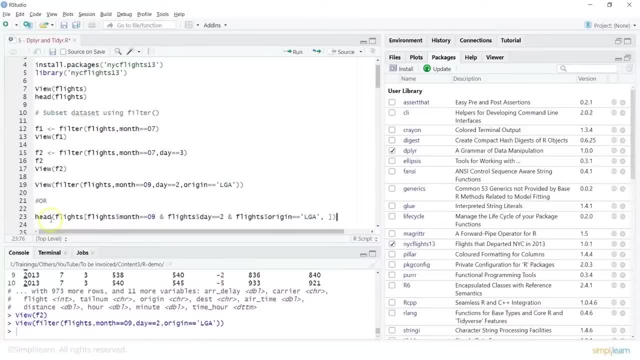 value. So in this way I can filter out specifically multiple values by specifying columns. Now, we could have done it in this way, we could have created a view, or we could have assigned this to a variable and then done a view on that, where we could have selected month. 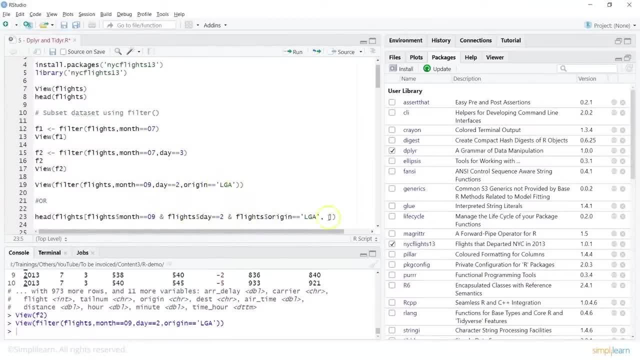 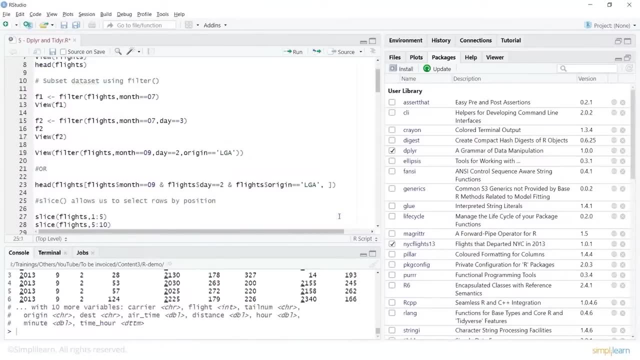 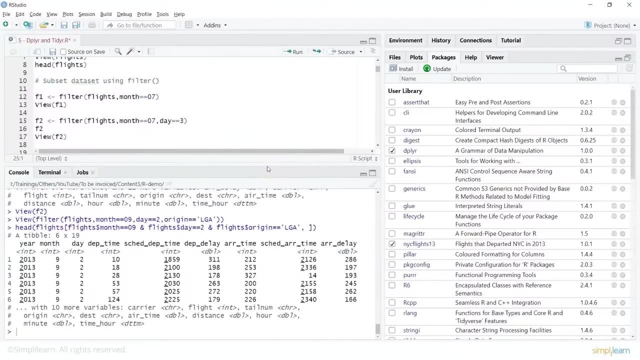 being day and origin, or you can be more specific in specifying all the columns. it makes the code more readable. so lets look at the values, and here you are looking at head, which shows me based on month, day, and then you can look for further columns for other variables, that is, origin being. 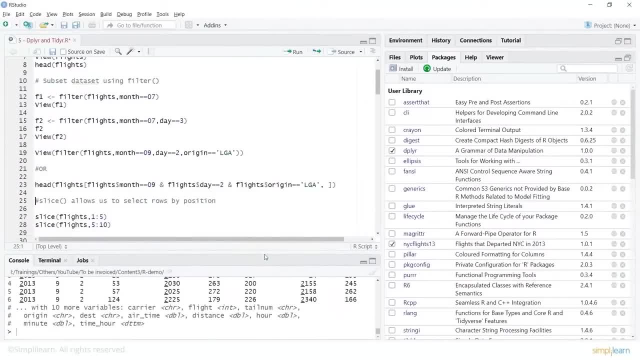 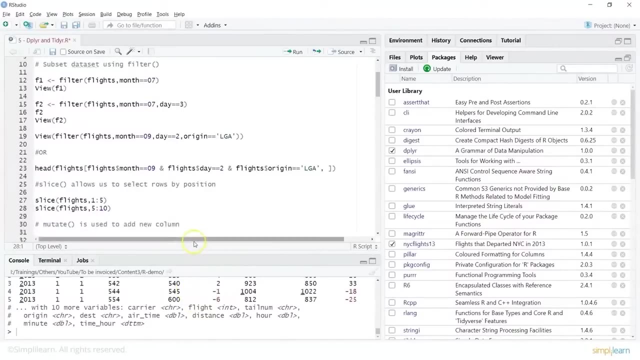 lga. Now what we can also do is we can do some slicing here to select rows by particular position. so I can say slice and I would want to look at rows 1 to 5, and I can do this. so you can always assign or look at the view of this. 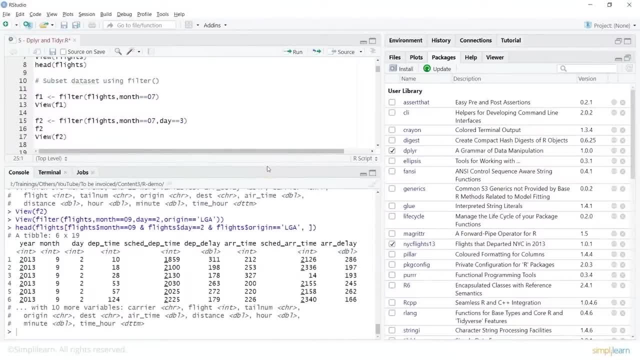 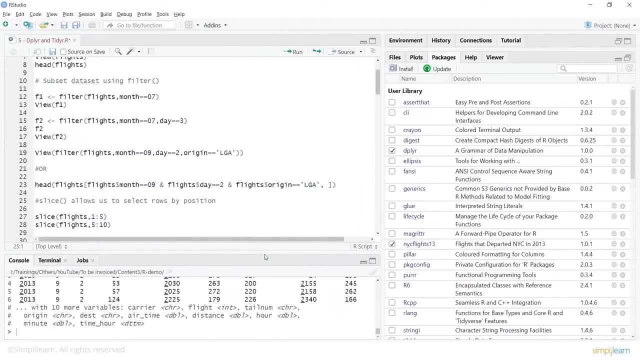 day, and then you can look for further columns for other variables. that is origin being lgea. now what we can also do is we can do some slicing here to select rows by particular position. so I can say slice and I would want to look at rows 1 to 5. 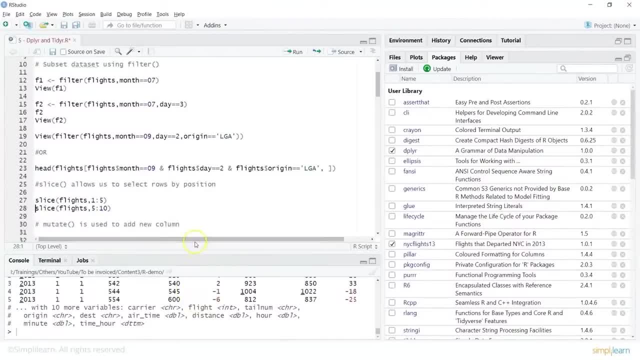 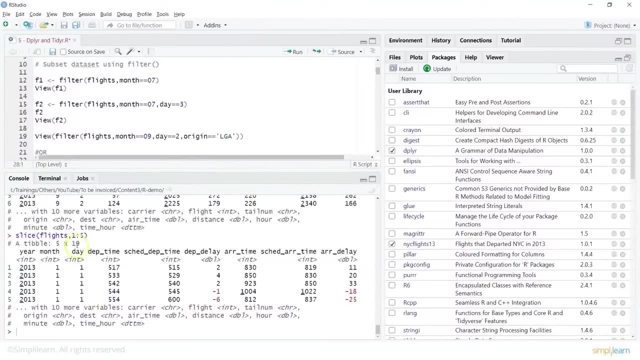 and I can do this, so you can always assign or look at the view of this I can just do here. so when I did a slice- 1 is to 5- it shows me my entries for 1 to 5. now, similarly, we can do a slice. 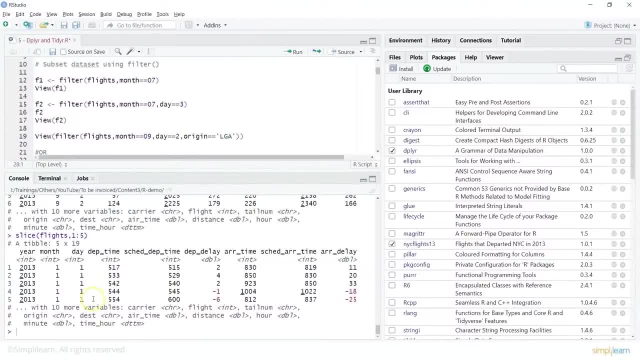 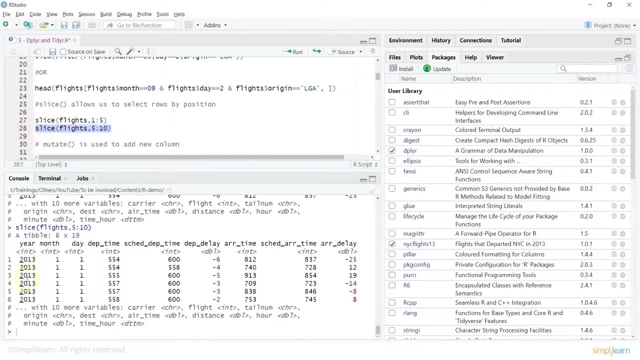 I can just do here. so when I did a slice, 1 is to 5, it shows me my entries for 1 to 5. now, similarly, we can do a slice 5 to 10, and now you are looking at 5 to 10 values. 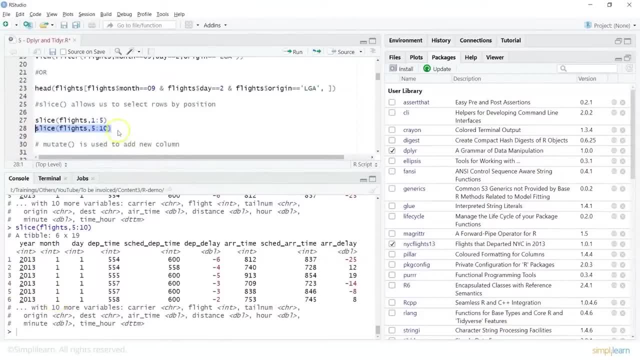 so you can always look at the complete data and then you can slice out particular data. now, mutate is usually a function which is used when you would want to apply some variable on a particular data set and then you would want to add it to your existing data. 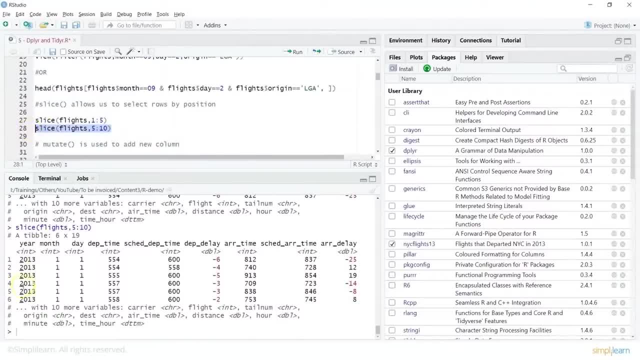 5 to 10, and now you are looking at 5 to 10 values, so you can always look at the complete data and then you can slice out particular data. now, mutate is usually a function which is used when you would want to apply some variable. 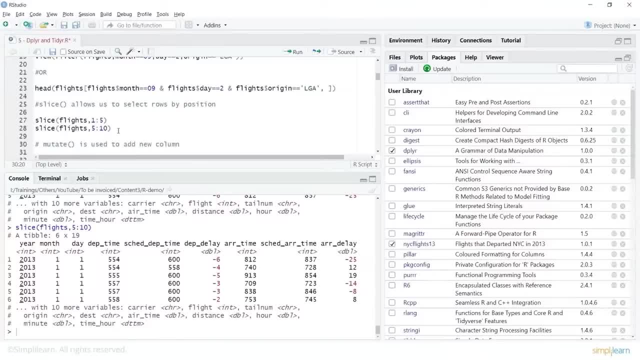 on a particular data set and then you would want to add it to your existing data frame, or you would want to add a new column. so this is where you use mutate, which is mainly used to add new variables. so let's see how you work on mutate. 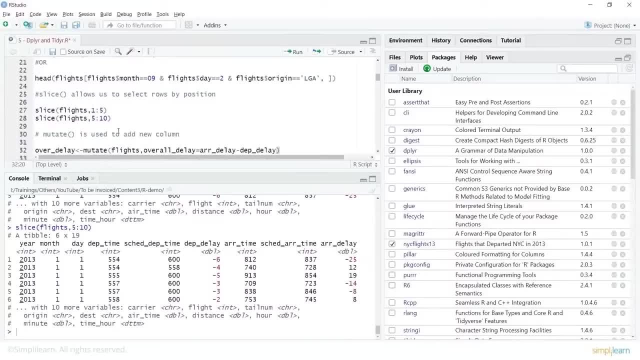 so it's pretty simple. so you create a variable over delay. now I would want to do a mutate so that it adds a new column. so I am selecting my data, which is flights, I will call the new column as overall delay and then basically I can look at. 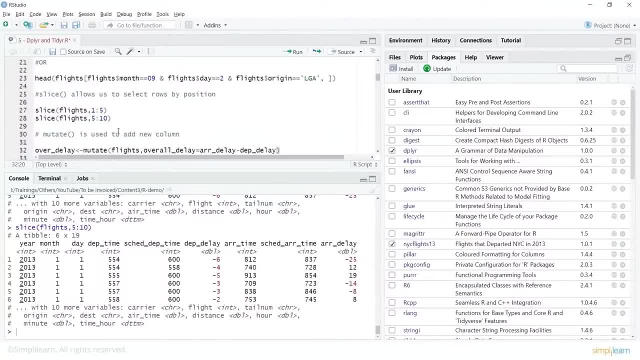 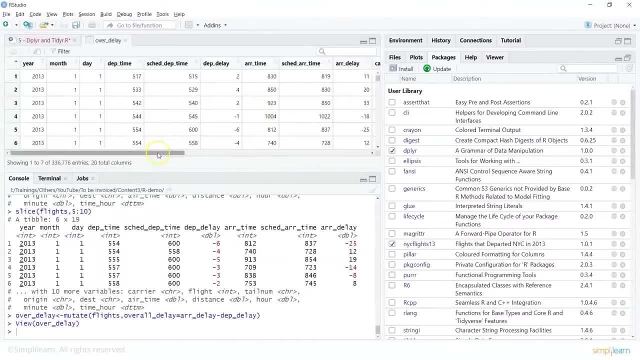 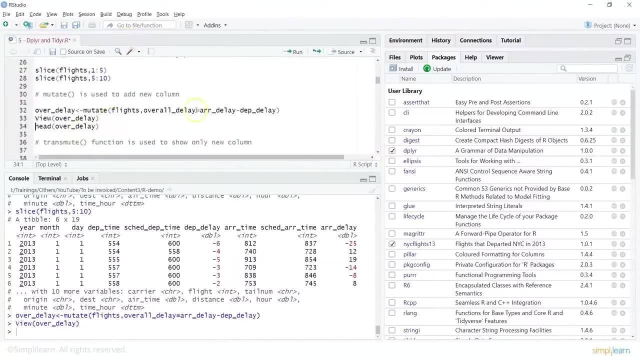 overall delay being arrival delay minus departure delay. so let's create this and let's look at view of this, which shows me- or which should show me- my new column, which is overall delay, which was not in my original data set. so you can anytime do a head. 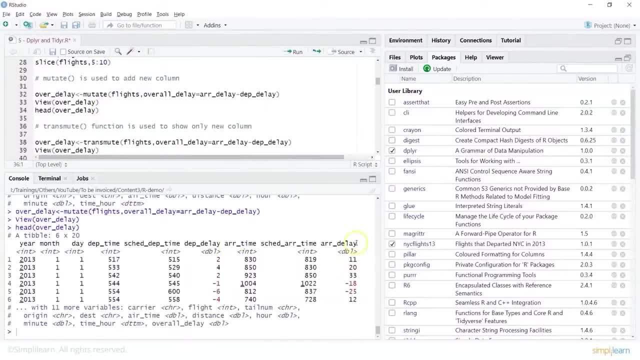 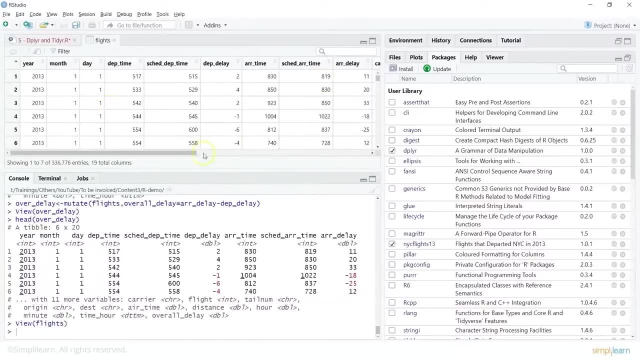 on this one to compare the value. so this one shows me arrival delay, and then there are many other variables. what you can also do is you can do a view and you could have just look at flights if you would want to compare. so you can look at the flights. 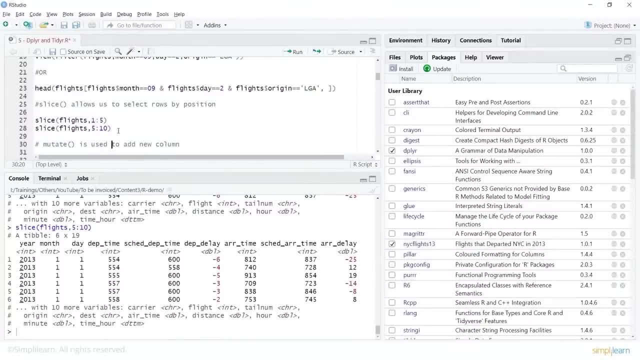 frame, or you would want to add a new column. so this is where you use mutate, which is mainly used to add new variables. so let's see how you work on mutate. so it's pretty simple. so you create a variable over delay. now I would want to do a mutate so that it adds: 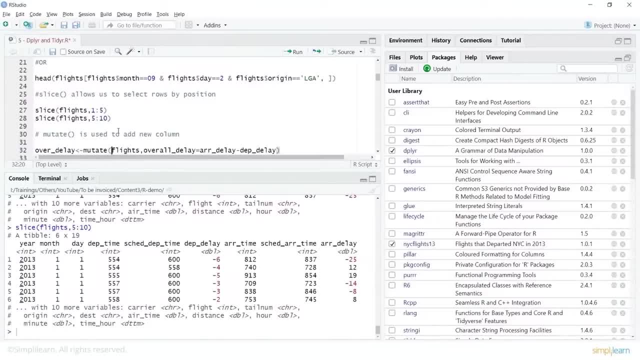 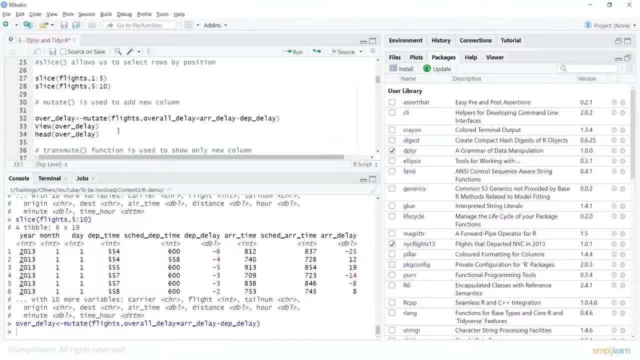 a new column. so I am selecting my data, which is flights, I will call the new column as overall delay and then basically I can look at overall delay being arrival delay minus departure delay. so let's create this and let's look at view of this, which shows me. 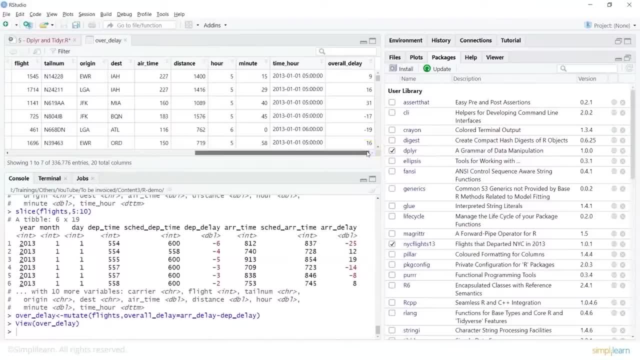 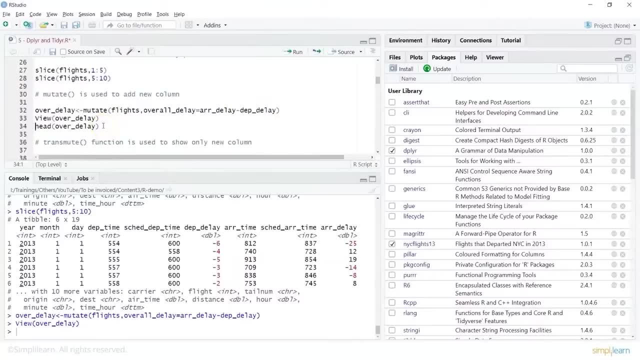 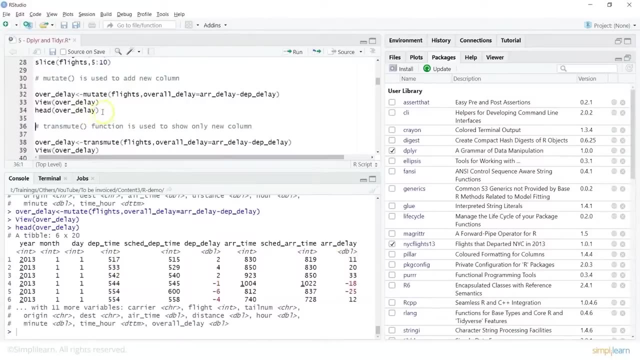 or which should show me my new column, which is overall delay, which was not in my original data set. so you can anytime do a head on this one to compare the value. so this one shows me arrival delay. and then there are many other variables, what you can also. 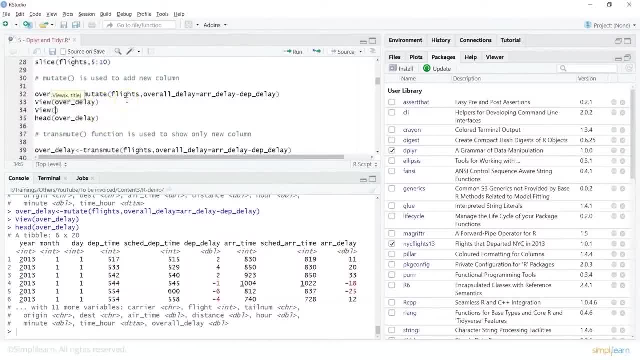 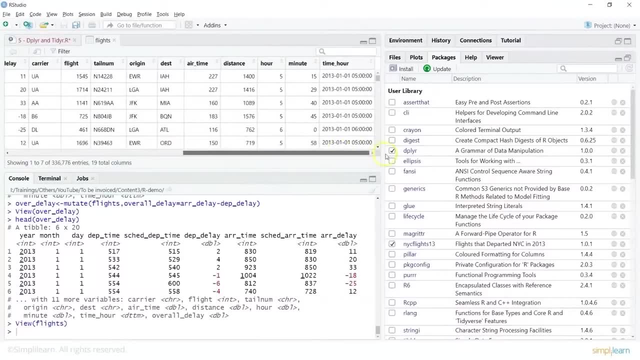 do is you can do a view and you could have just look at flights if you would want to compare. so you can look at the flights and this one would not have any overall delay column. so it basically shows me 19 columns, only what we see here and 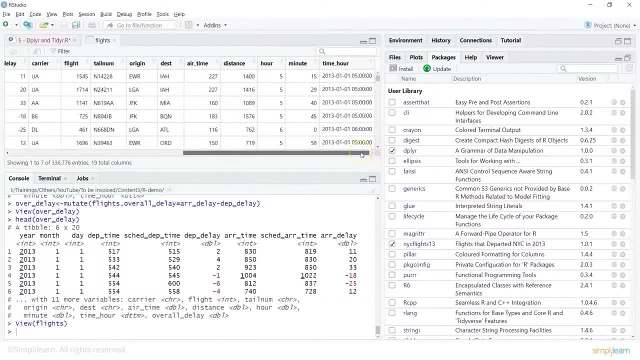 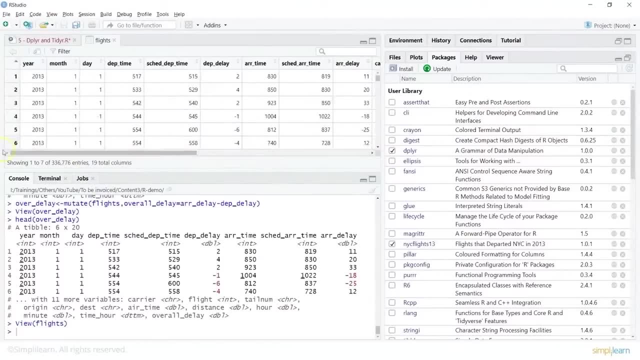 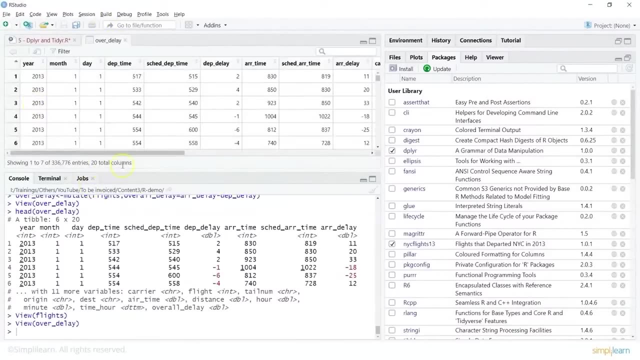 and this one would not have any overall delay column. so it basically shows me 19 columns- only what we see here, and if you do a view on overall delay, then that basically shows me 20 columns. so we know that the new column has been added to. 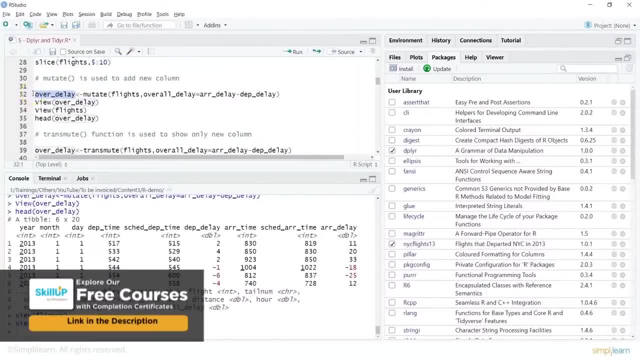 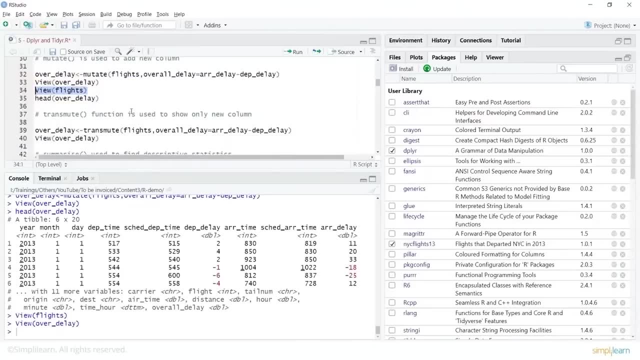 this overall delay. so if you would want to work with 20 columns, you will use overall delay. if you would want to work with your original data set, you will use flights. now you can also use a transmute function, which is used to show only the new column. 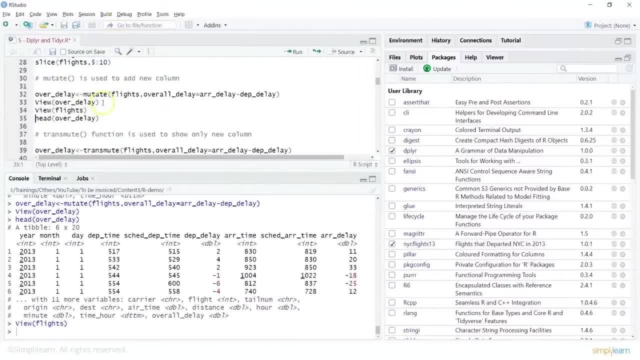 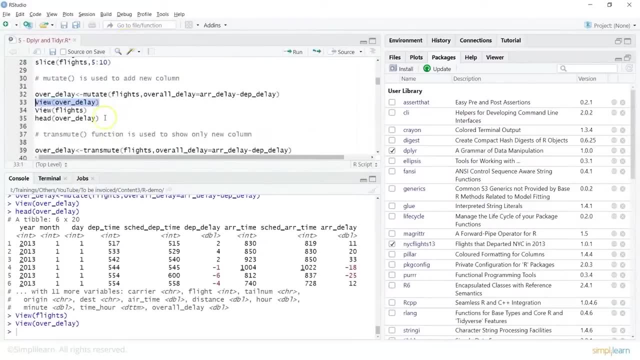 if you do a view on overall delay, then that basically shows me 20 columns. so we know that the new column has been added to this overall delay. so if you would want to work with 20 columns, you will use overall delay if you would want to work with your original data. 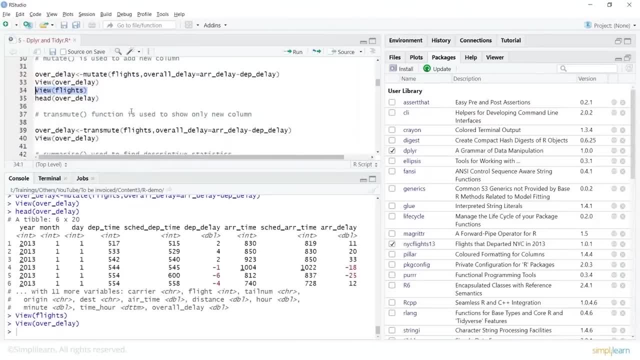 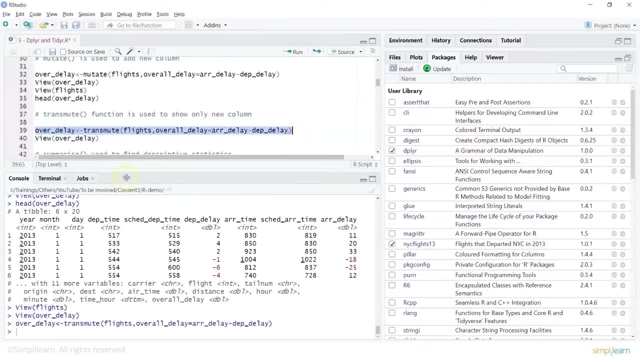 set, you will use flights. now you can also use a transmute function which is used to show only the new column. so we can do a overall delay and at this time we will say transmute, we will say flights, overall delay. the computation remains same, but at this time, if I look at 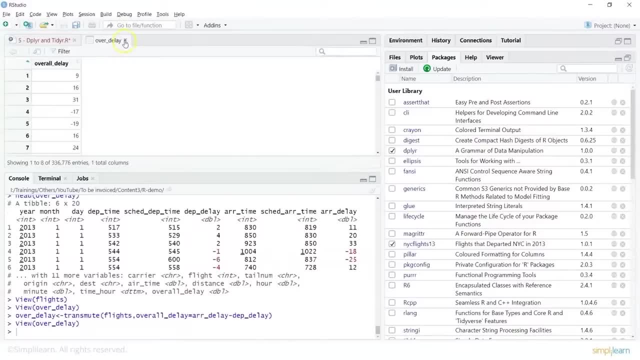 view on overall delay. it only shows me the new column, so sometimes we may want to compute result based on two ways, or two variables or two columns, and just look at the new value and then we can decide if we would want to add it to our existing structure now. 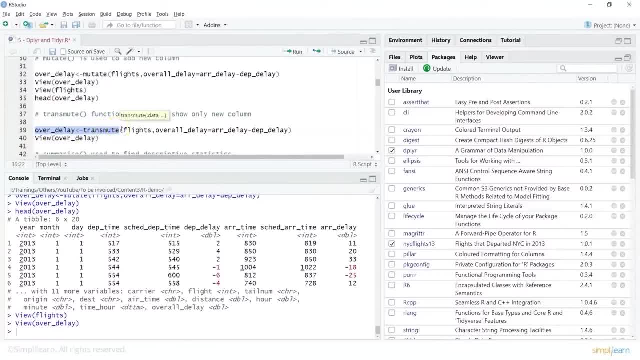 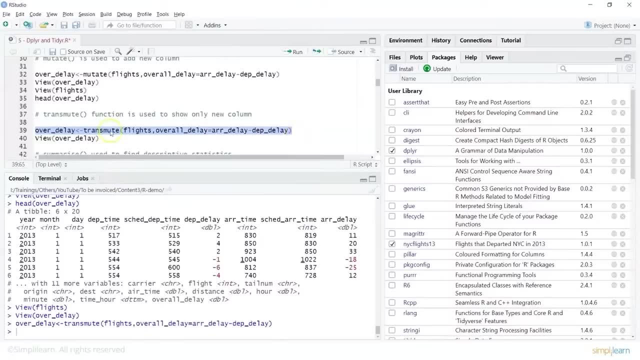 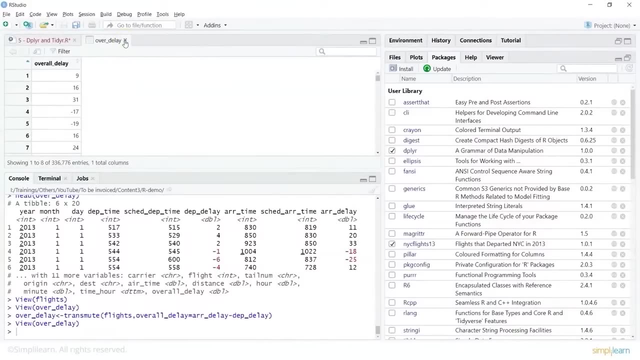 so we can do a overall delay and at this time we will say transmute, we will say flights, overall delay. the computation remains same. but at this time if I look at view on overall delay it only shows me the new column. so sometimes we may want to compute. 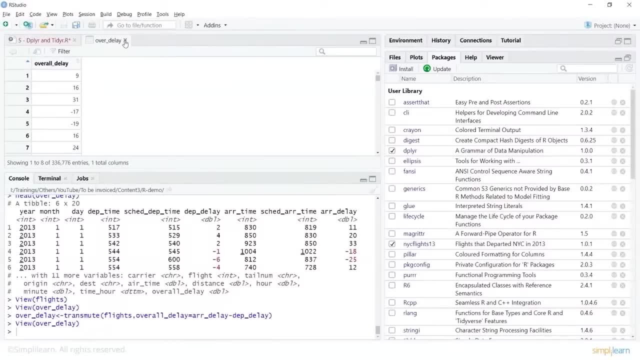 result based on two variables or two columns, and just look at the new value and then we can decide if we would want to add it to our existing structure. now you can also use summarize, and summarize basically helps us in getting a summary based on certain criteria, so we can always do a 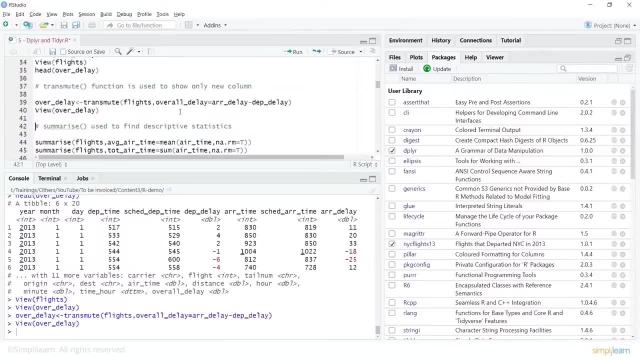 summarize. and what we can do is we can look at our data and we can say on what basis we would want to summarize this particular data. so we can do a summarize function. now summarize on flights: I will say average airtime and I would want to calculate. 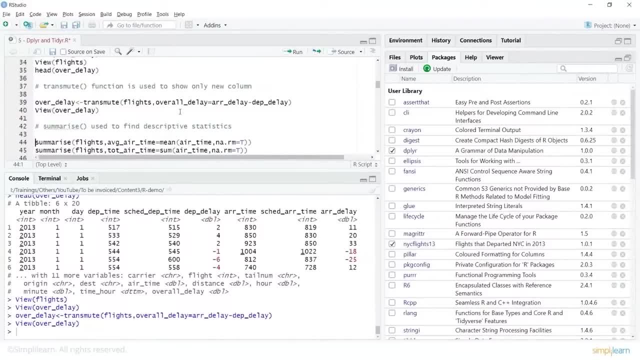 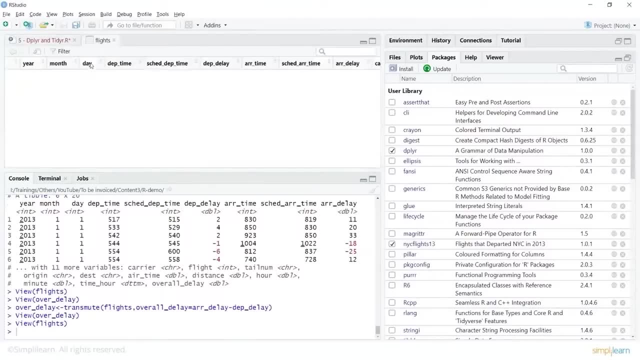 an average. so for that I am using an inbuilt function called mean. I will do that on airtime column. so let's look at flights once again and here we can see there is arrival time, not airtime. sorry, arrival time and we would want to do. 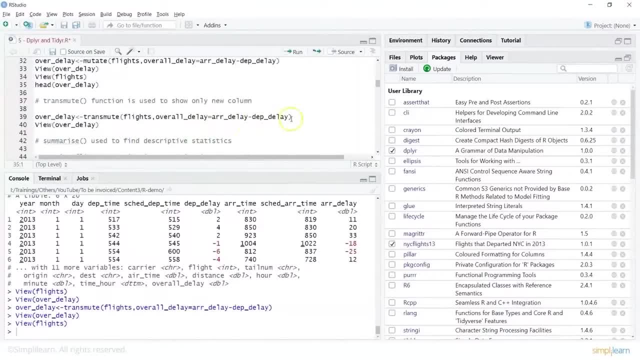 some average on this particular data. we would want to summarize this, so what I will do is I will use the summarize function. I will say average airtime and this one I will look at mean of airtime. so let's see if there is a airtime column. 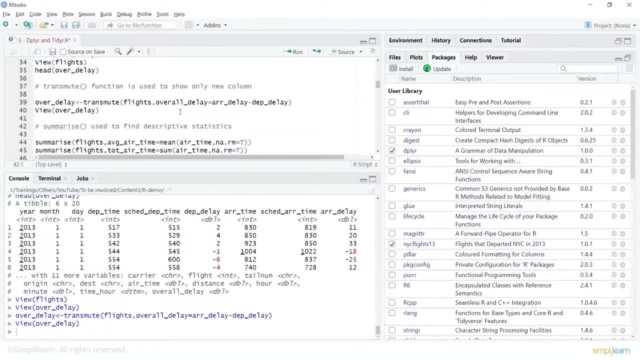 you can also use summarize, and summarize basically helps us in getting a summary based on certain criteria. so we can always do a summarize, and what we can do is we can look at our data and we can say on what basis we would want to summarize this particular data. so 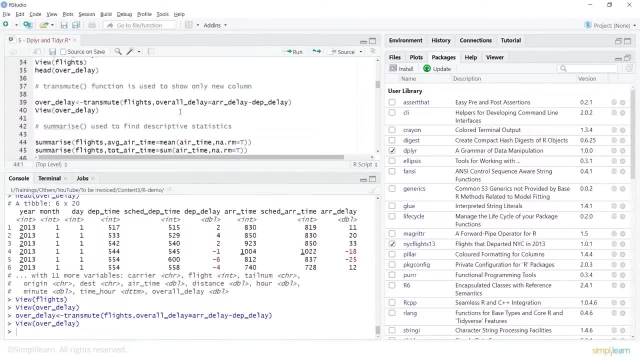 we can do a summarize function. now, summarize on flights. I will say average airtime and I would want to calculate an average. so for that I am using inbuilt function called mean. I will do that on airtime column. so let's look at flights once again and here 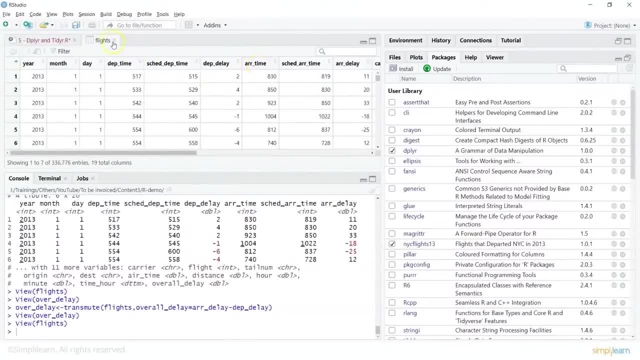 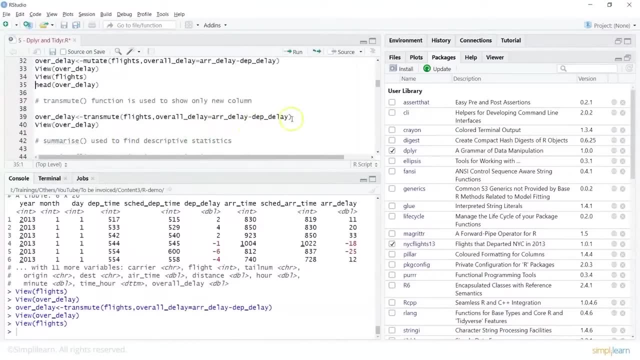 we can see there is arrival time, not airtime- sorry, arrival time- and we would want to do some average on this particular data. we would want to summarize this. so what I will do is I will use the summarize function, I will say average airtime and this one. 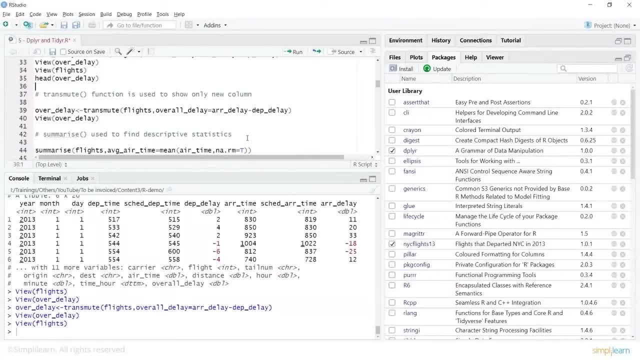 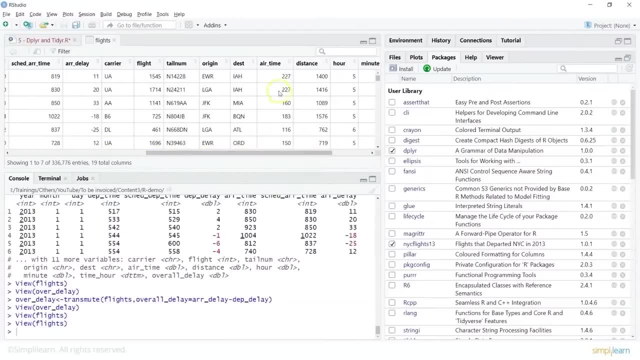 I will look at mean of airtime. so let's see if there is a airtime column. I might be. let's look at this one arrival delay and yes, we have an airtime. so we were actually looking at summarizing based on airtime, not the 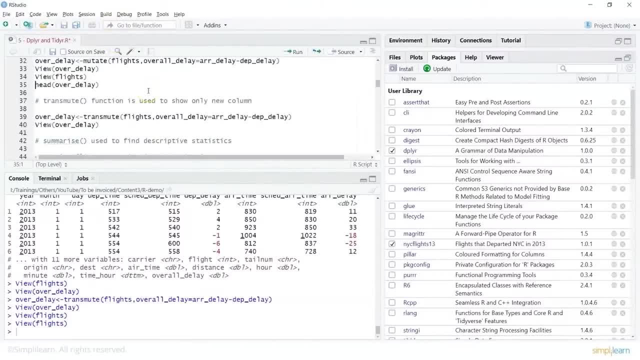 arrival time. so airtime is how much time it takes in air for this particular flight, and we will want to use the trans summarize function, not the transmute. so summarize flights: average airtime and this one: we will calculate the mean of average airtime and I will also do a 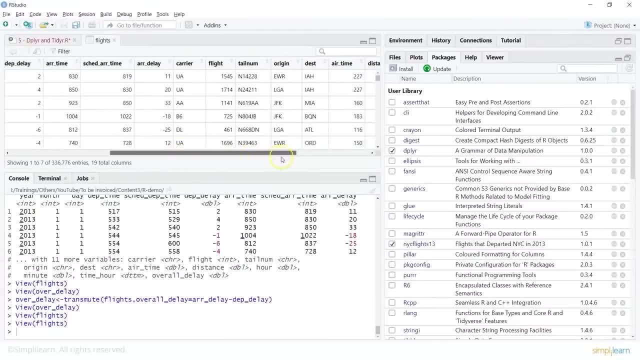 I might be. let's look at this: one arrival delay and, yes, we have an airtime. so we were actually looking at summarizing based on airtime, not the arrival time. so airtime is how much time it takes in air for this particular flight and we will want to use 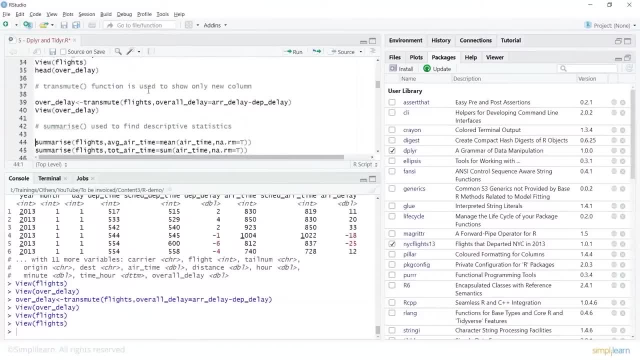 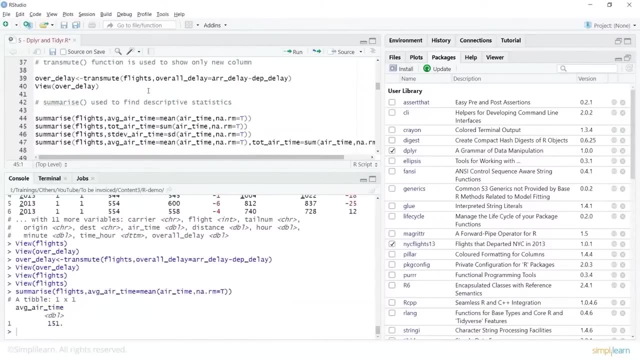 the trans summarize function, not the transmute. so summarize flights: average airtime and this one. we will calculate the mean of average airtime and I will also do a any removal, which is: I am saying true, so let's do this. and that basically shows me the average airtime is 151. 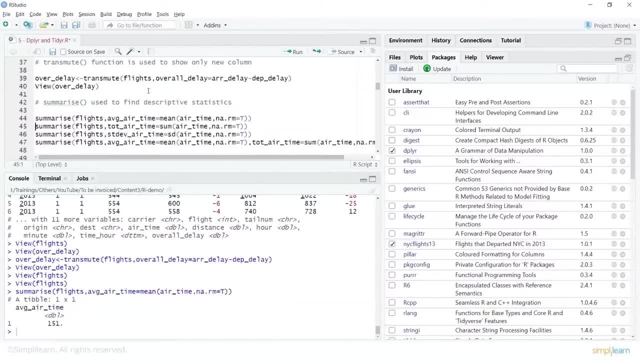 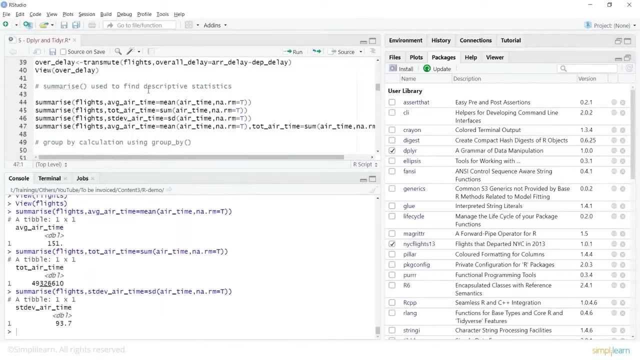 any removal, which is I am saying true. so let's do this. and that basically shows me. the average airtime is 151. I can also do a total airtime where I am doing a summation of values, or I can get the standard deviation or I can basically. 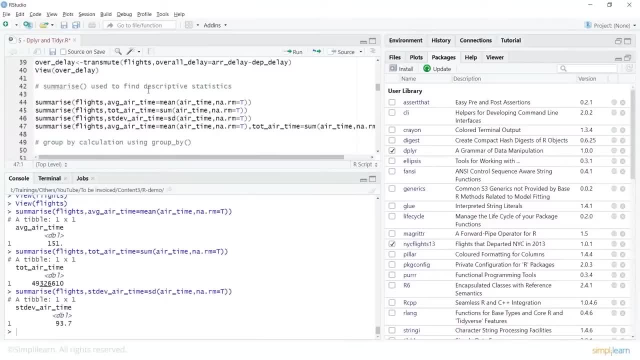 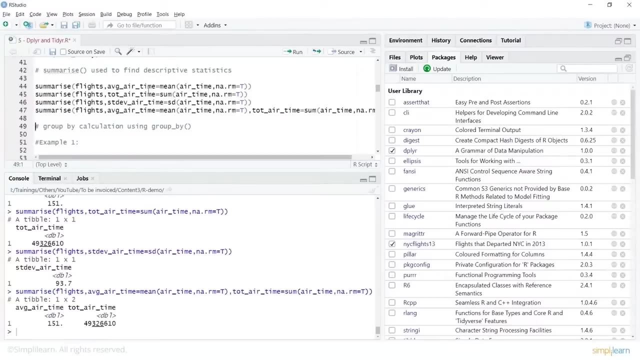 get multiple values, such as mean, I can say total airtime, where I am doing a summation, and then I can look at other values, which is if you would want to put in standard deviation here. you could do that. so let's look at the result of this summarize. 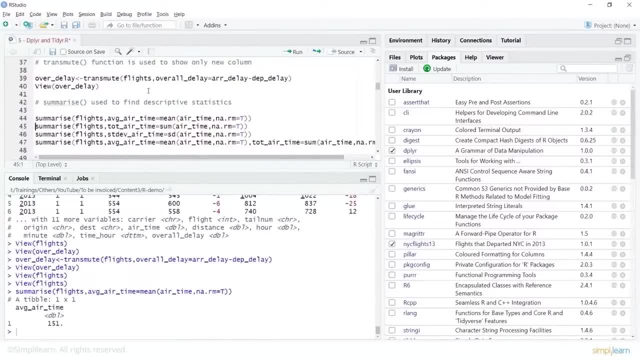 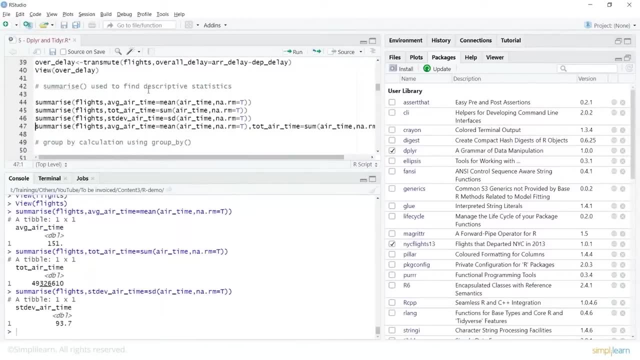 I can also do a total airtime where I am doing a summation of values. or I can get the standard deviation, or I can basically get multiple values, such as mean I can say total airtime where I am doing a summation, and then I can look at other values. 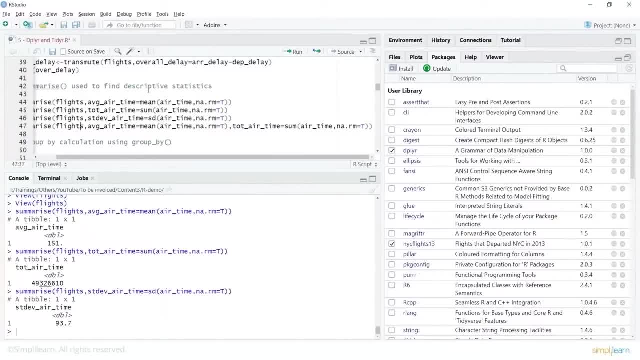 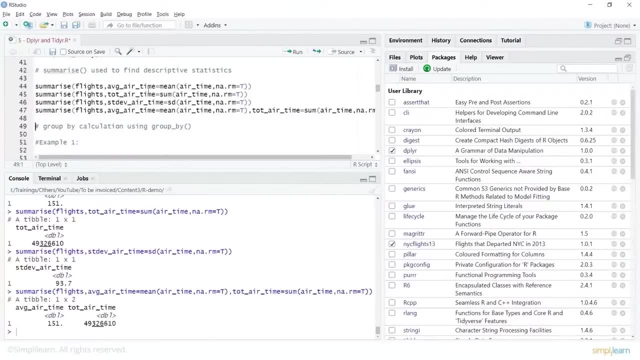 which is, if you would want to put in standard deviation here, you could do that. so let's look at the result of this summarize, and this basically allows me to get some useful information which is summarized based on a particular function, such as mean, some standard deviation or all three of them. 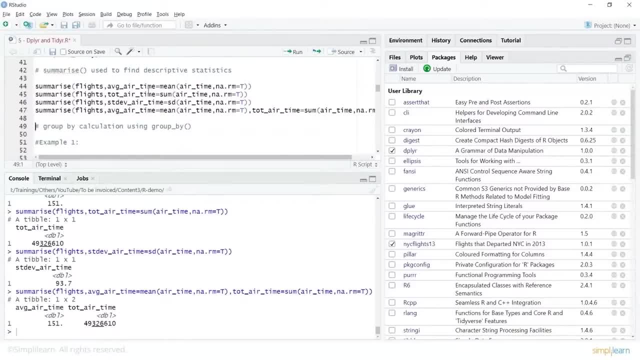 now let's look at grouping by. so sometimes we may be interested in summarizing the data by groups, and that's where we use the group by function. so we can always use the group by clause. now, here we are taking a different data set. so we will say, for example: 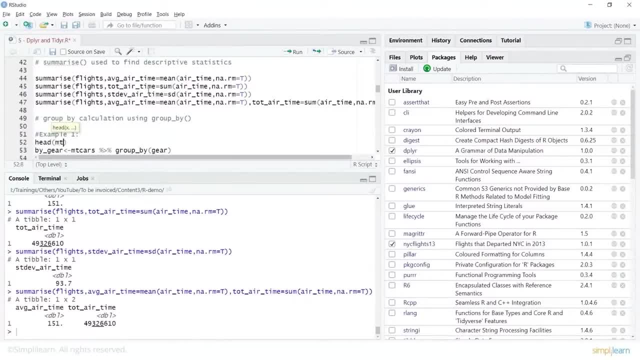 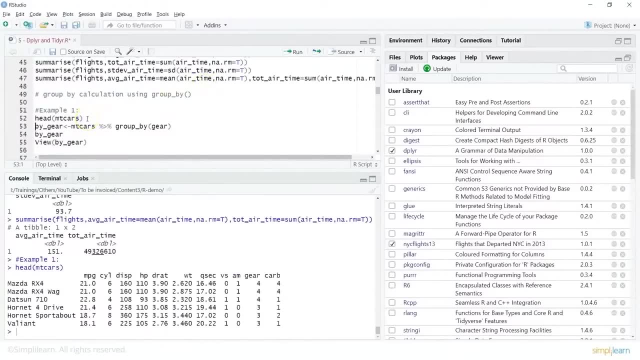 let's look at head of empty cars and that is basically my data set on empty cars. now that shows me the model of the car, it shows me mileage, cylinder power and your horsepower and various other characteristics or variables in this particular data set. so here we can say: 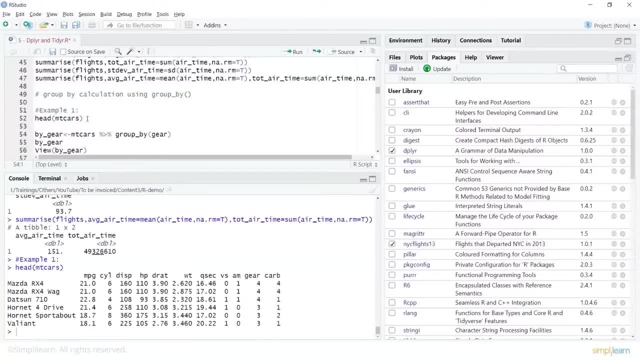 let's do a grouping by gear. so there is a column called gear, so I will call it by gear. I will look at my data set and then what I am using here, which you see with these percentage and greater symbol, is called piping, so that basically feeds. 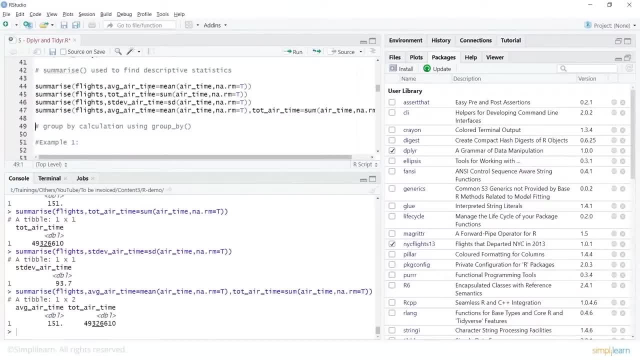 and this basically allows me to get some useful information which is summarized based on a particular function, such as mean, some standard deviation or all three of them. now let's look at grouping by. so sometimes we may be interested in summarizing the data by groups, and that's where we use. 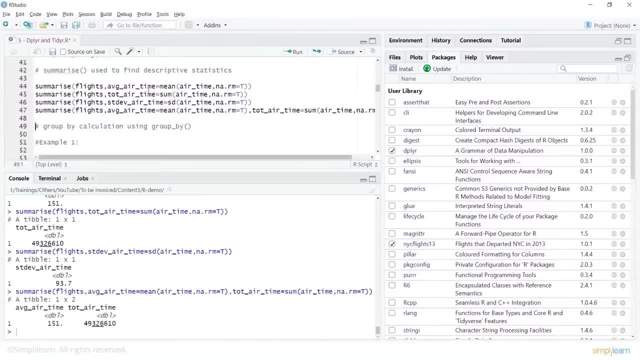 the group by function, so we can always use the group by clause. now here we are taking a different data set. so we will say, for example, let's look at head of empty cars, and that is basically my data set on empty cars. now that shows me the model of the car. 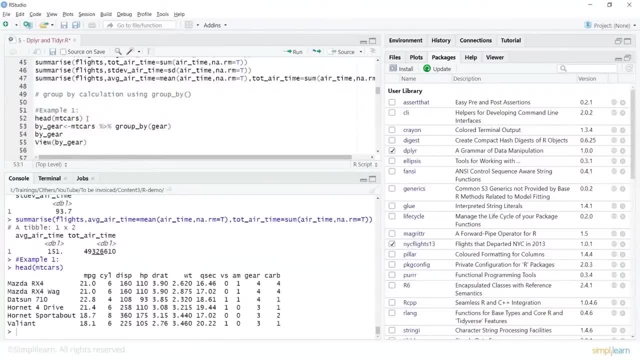 it shows me mileage, cylinder power and your horse power and various other characteristics or variables in this particular data set. so here we can say: let's do a grouping by gear. so there is a column called gear, so I will call it by gear. I will look at. 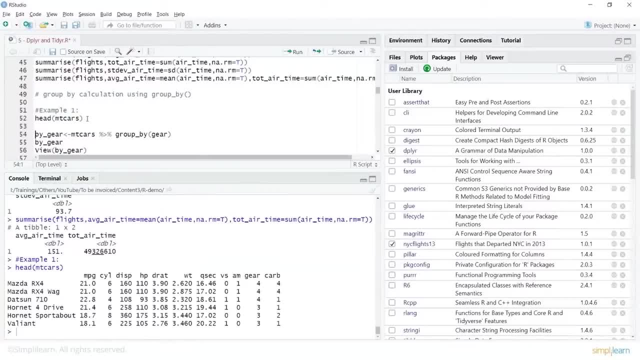 my data set and then what I am using here, which you see with these percentage and greater symbol, is called piping, so that basically feeds your previous data frame into next one. so this is sometimes useful and you can get this by just saying control, shift and M and you. 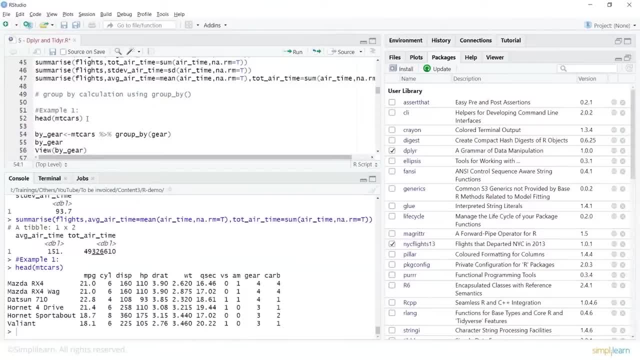 can then use this. so we are going to have piping, so I am saying empty cars. now this is my original data set where I did a head, or I could have done a view on this one, if you would want to see it in a more readable format. 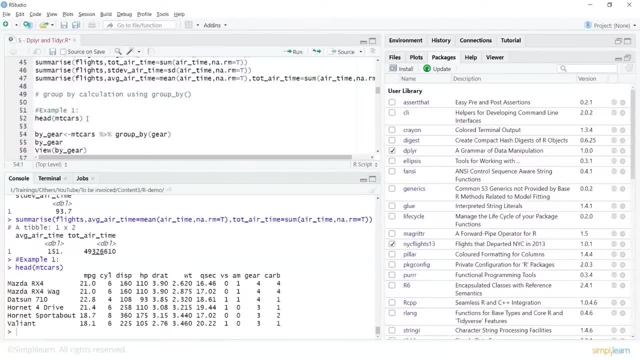 your previous data frame into next one. so this is sometimes useful and you can get this by just saying control, shift and M and you can then use this. so we are going to have piping, so I am saying empty cars now. this is my original data set where I did a head. 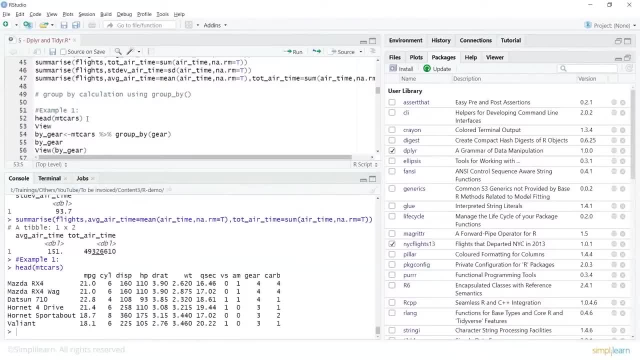 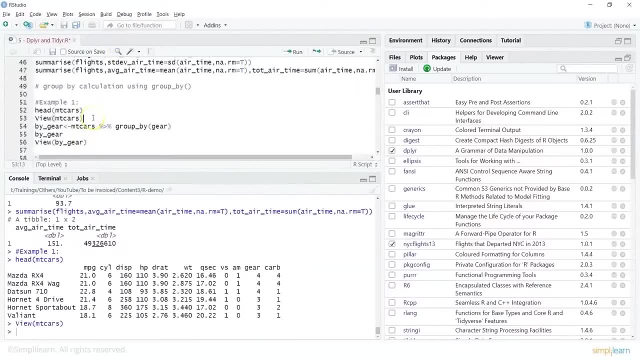 or I could have done a view on this one if you would want to see it in a more readable format. and that basically shows me the data. so we are using a different data set, so I want to group it by the gear column. so I am going to call it by gear. 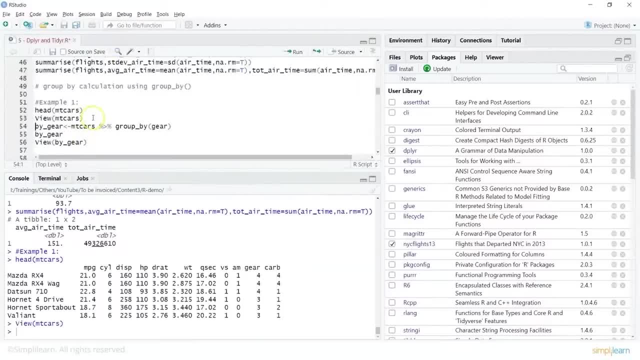 and that basically shows me the data. so we are using a different data set, so I want to group it by the gear column. so I am going to call it by gear and this one takes my data, that is empty cars. I am using the piping and then I am. 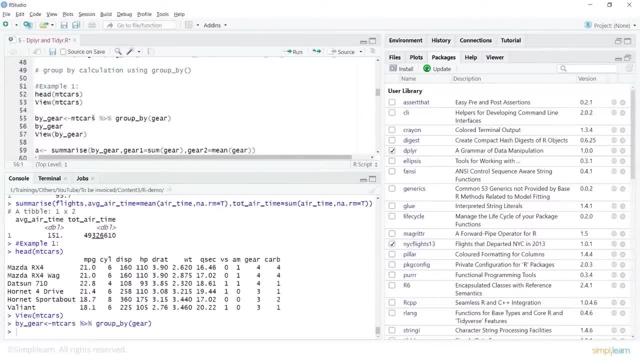 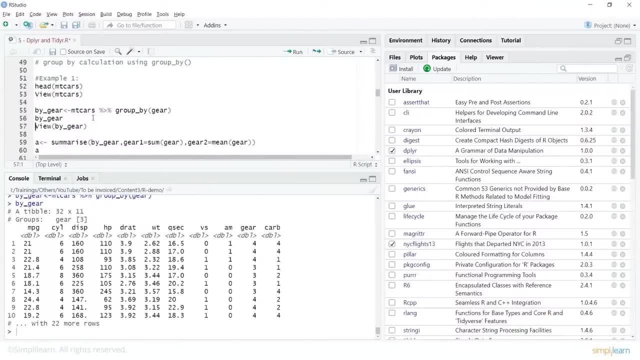 saying: group the data based on gear column. that's done. now let's look at the value of by gear or you can always do a view. so remember, whenever you are doing a group by, it is giving you a internal object where your data is grouped based on a particular 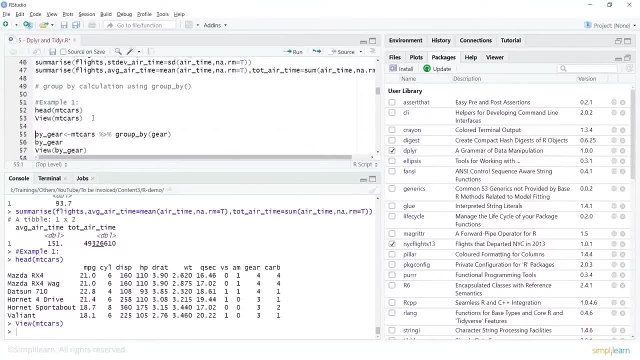 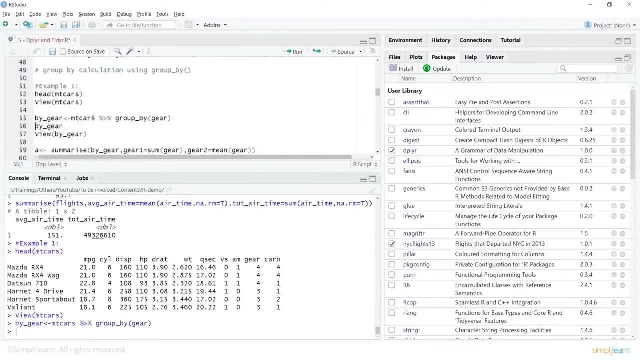 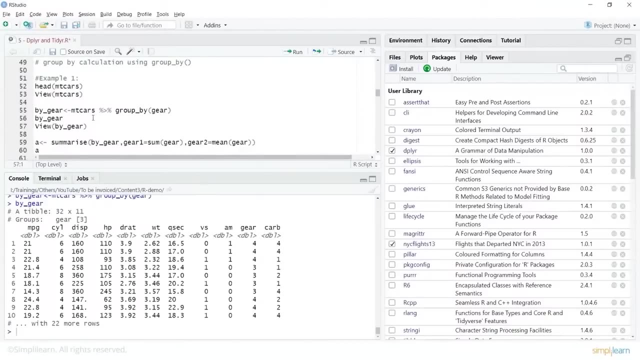 and this one takes my data, that is, empty cars. I am using the piping and then I am saying: group the data based on gear column. that's done. now let's look at the value of by gear, or you can always do a view. so remember whenever you are doing a group by. 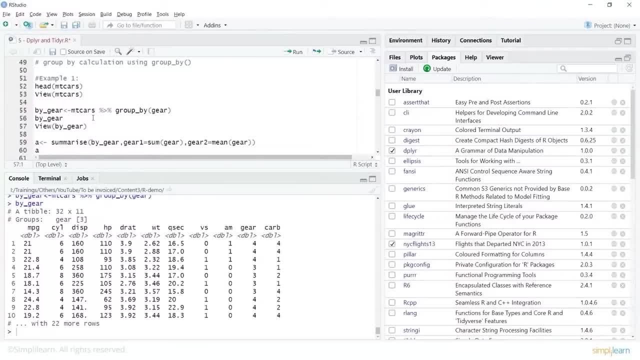 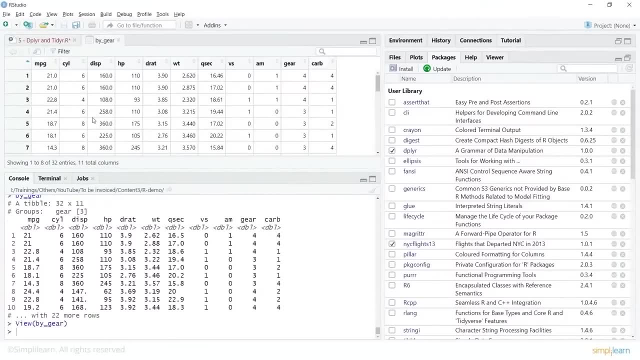 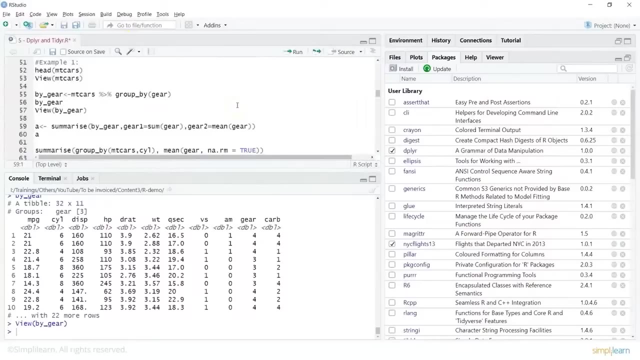 it is giving you a internal object where your data is grouped based on a particular column. so we can look at the values here you can do a view that shows you your data group based on a particular column. now I can again use the summarize function where I would want to now work on the new one. 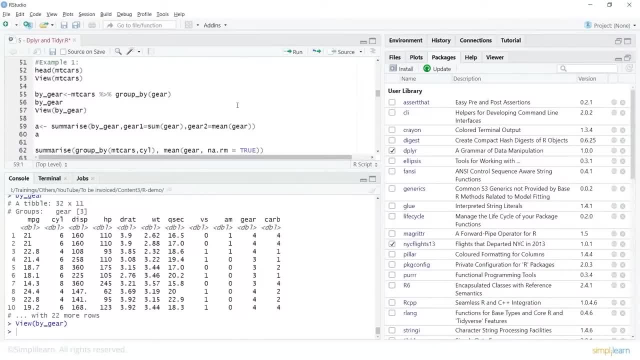 where it was grouped based on gear. so I am doing a summarize and here I am going to say gear 1, which will be having the value of summation on the gear column, and then I am saying gear 2, which is mean. well, you could give some meaningful names to this. 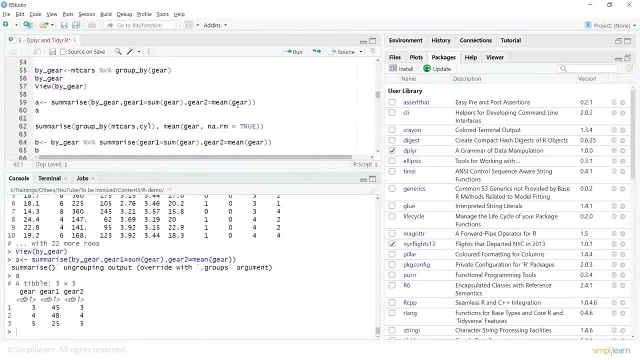 and let's look at the value of this one, where we are basically now looking at the values, which is sum and mean values based on the gear. similarly, we can use- look at different example- so we can say, by gear- and I am again using piping, but earlier we had taken gear- 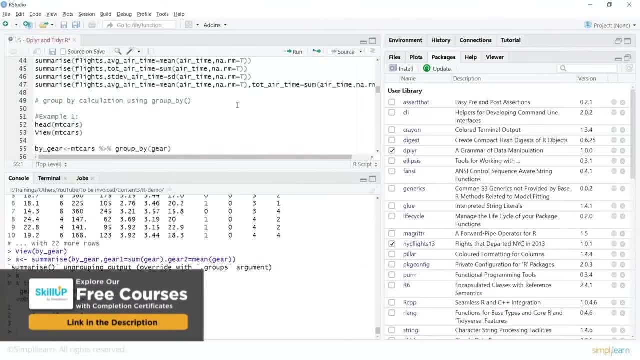 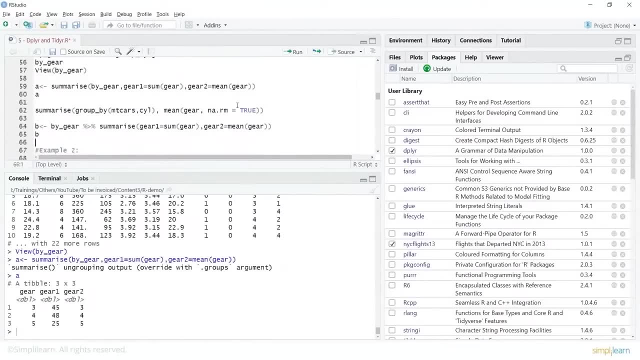 we had grouped the data and we called it by gear. so we took our original data set, empty cars. but now, within this particular data which was grouped by gear, I will take this data set, I will use the piping and I will summarize it where I am saying: 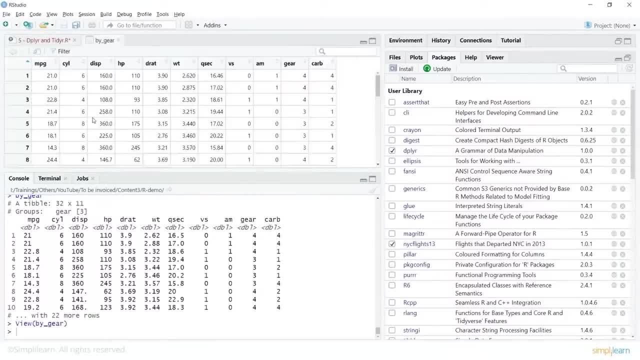 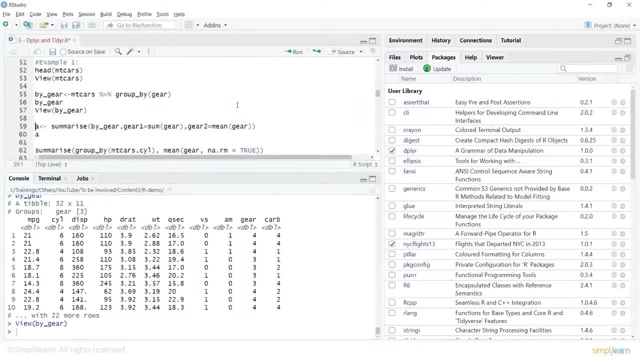 column so we can look at the values. here you can do a view that shows you your data group based on a particular column. now I can again use the summarize function where I would want to now work on the new one where it was grouped based on gear. so I am doing a summarize. 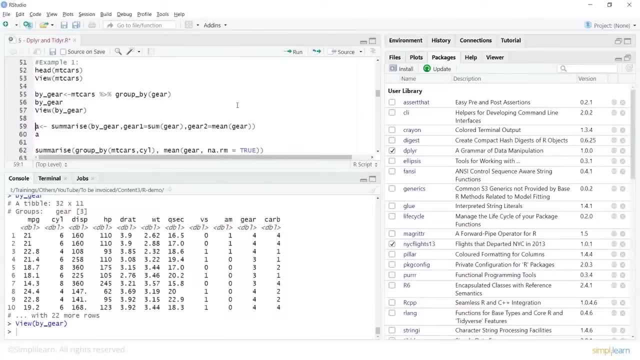 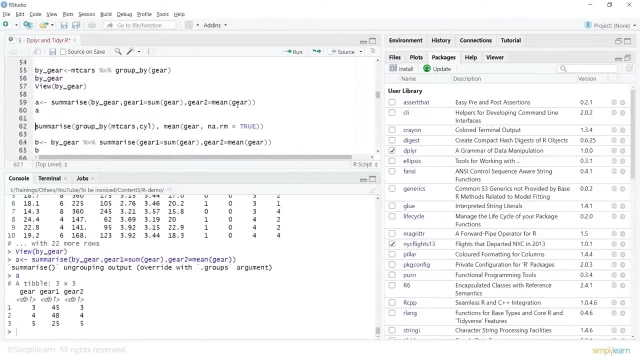 and here I am going to say gear one, which will be having the value of summation on the gear column, and then I am saying gear two, which is mean- well, you could give some meaningful names to this. and let's look at the value of this one, where 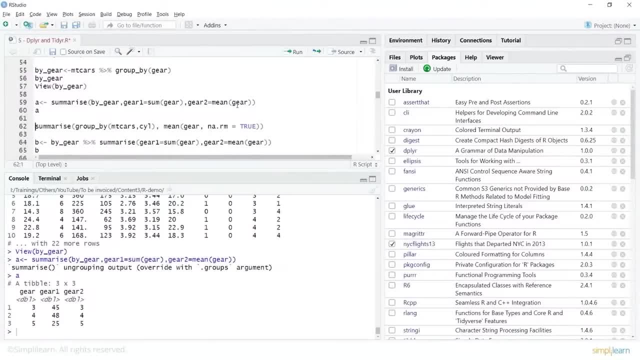 we are basically now looking at the values, which is sum and mean values based on the gear. similarly, we can use- look at different example, so we can say by gear- and I am again using piping, but earlier we had taken gear, we had grouped the data and we called it by gear. so we took 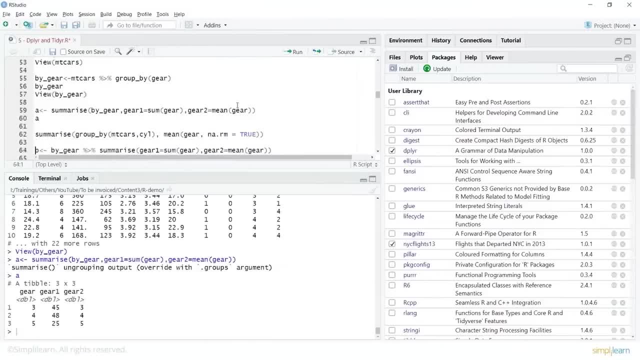 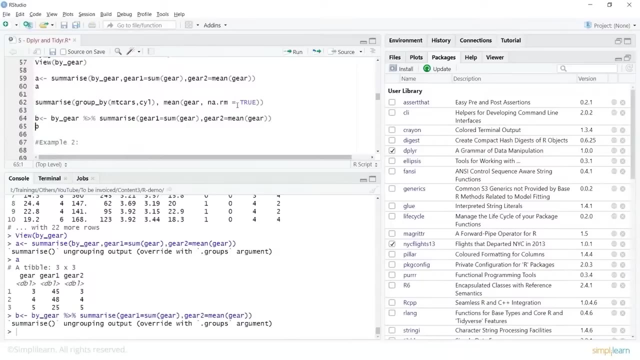 our original data set, empty cars. but now, within this particular data, which was grouped by gear, I will take this data set, I will use the piping and I will summarize it where I am saying, within this particular data set, I would want to get the sum or I would want to get the mean. 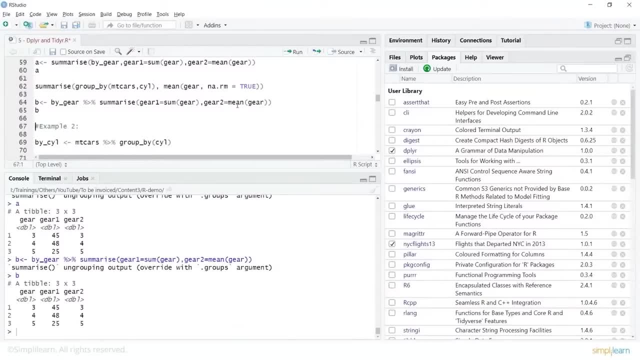 and then you can look at the values. so what you are doing is you are either looking at your original data set or you are looking at the data which was already grouped, and then you can look at the values. now here, what we can do is we can group by cylinder, say might. 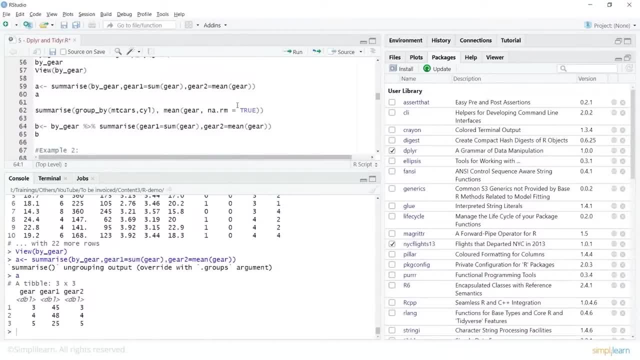 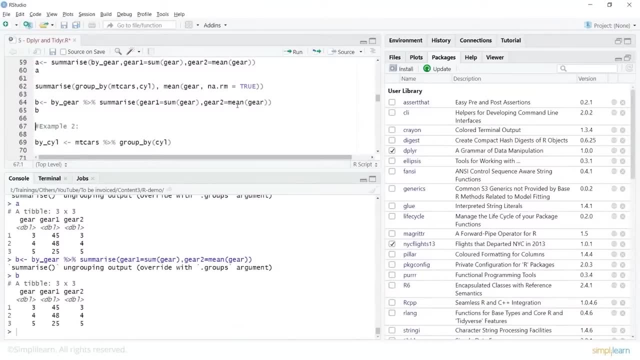 within this particular data set. I would want to get the sum, or I would want to get the mean, and then you can look at the values. so what you are doing is you are either looking at your original data set or you are looking at the data which was already grouped. 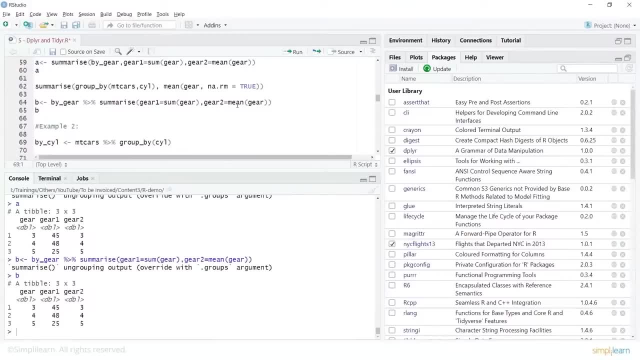 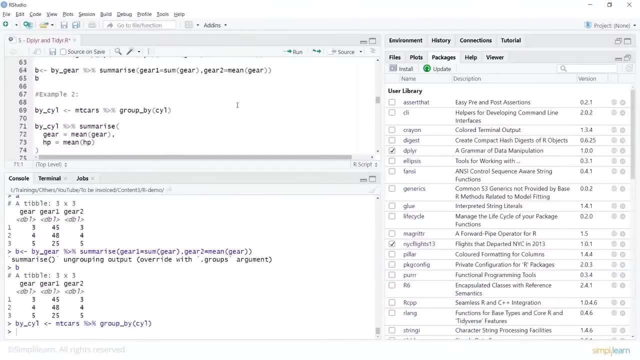 and then you can look at the values. now, here, what we can do is we can group by cylinder, say, might be you are interested in looking at data which is summarized based on the cylinder column. you can do that and then for this by cylinder. I am doing a piping. 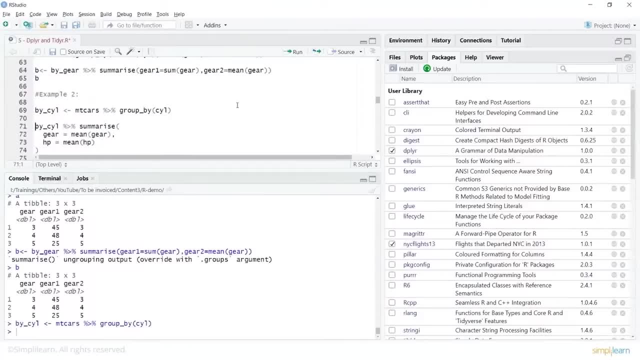 be you are interested in looking at data which is summarized based on the cylinder column. you can do that and then for this by cylinder, I am doing a piping where I am using the summarized function and summarizing will then be done based on the mean values of the gear column or the horse. 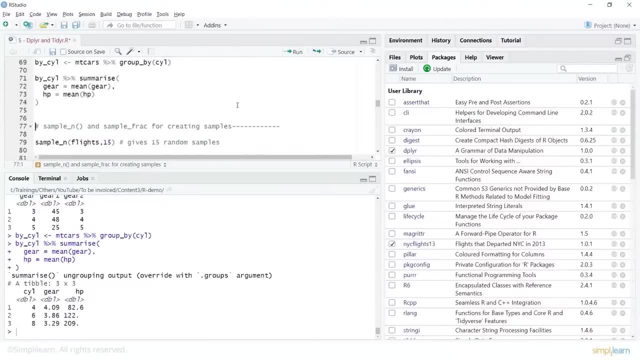 power. so lets do this, and then you can basically look at the value. at any point you may want to look at the data set again, so just do a head and you can look at what is the value contain, and by cylinder or by gear. and do a head and 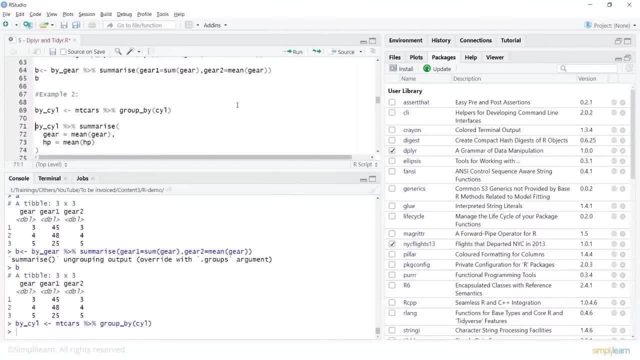 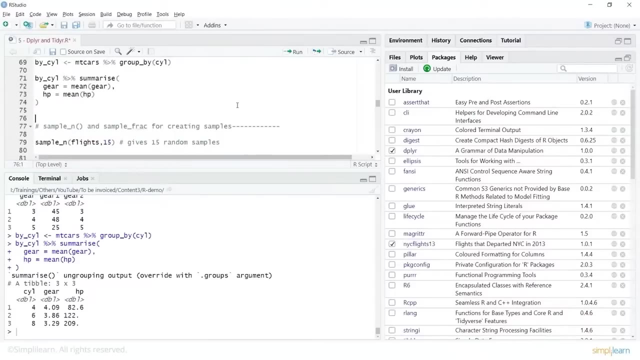 where I am using the summarize function, and summarizing will then be done based on the mean values of the gear column or the horse power. so let's do this, and then you can basically look at the value at any point. you may want to look at the data set again. 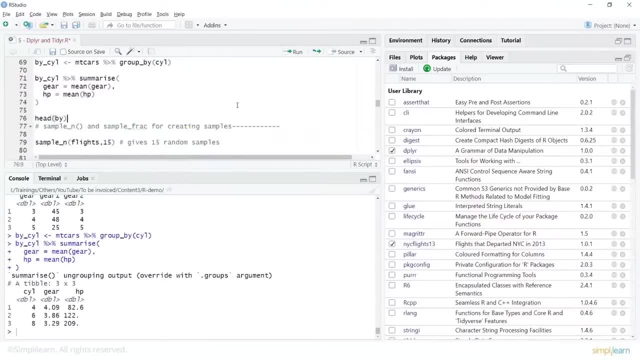 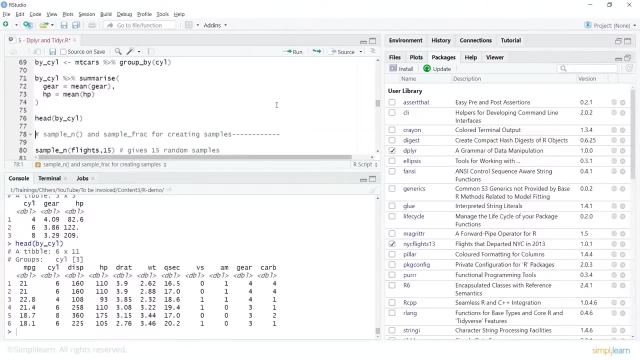 so just do ahead and you can look at what does the value contain, and by cylinder or by gear, and do ahead and it gives you the value. so you can always do some summarizing or grouping in these ways. now here we are going to use sample underscore n function. 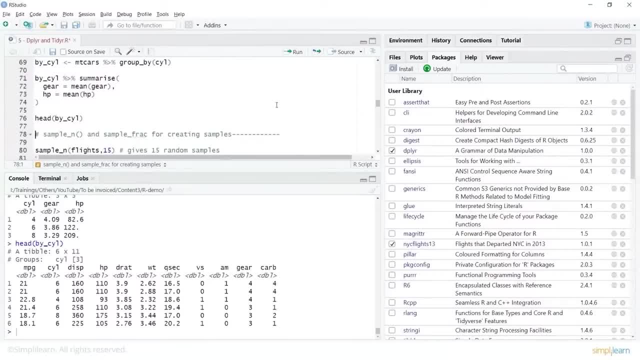 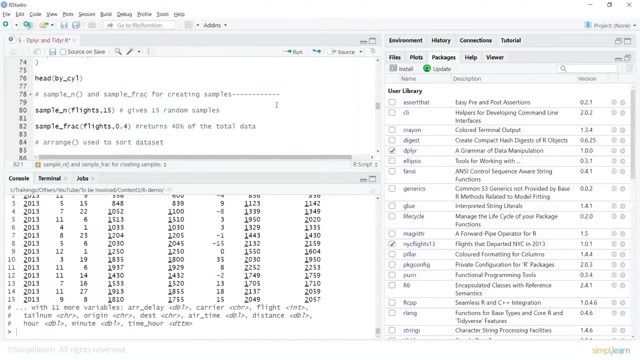 and sample underscore fraction for creating samples. so for this, let's take the flights data set again and we would want to get fifteen random values. now that is done and it shows me fifteen rows with some random values from the data. what you can also do is you can do a portion of data. 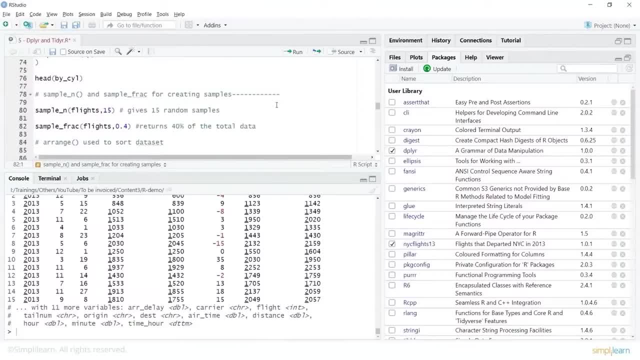 by using sample underscore fraction, and here I will say flights, I will say point four, which will return forty percent of the total data. so this can be useful when you are building your machine learning, where you would want to split your data into training and test might be you are interested in. 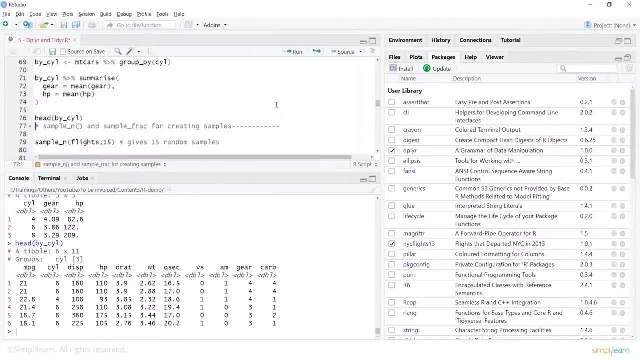 it gives you the value, so you can always do some summarizing or grouping in these ways. now, here we are going to use sample underscore n function and sample underscore fraction for creating samples. so for this, lets take the flights data set again and we would want to get 15 random. 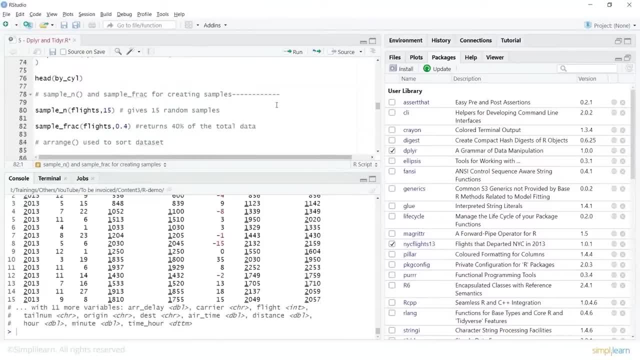 values. now that is done and it shows me 15 rows with some random values from the data. what you can also do is you can do a portion of data by using sample underscore fraction, and here I will say flights, I will say .4, which will return. 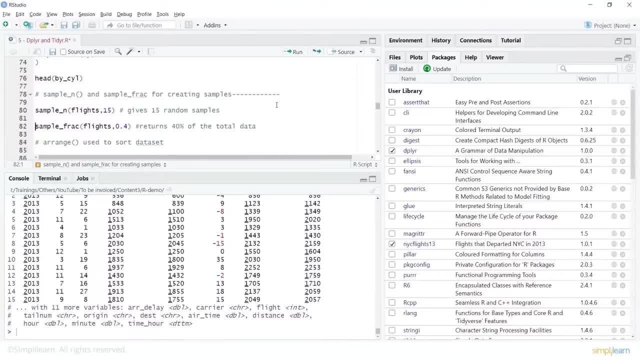 40% of the total data, so this can be useful when you are building your machine learning. where you would want to split your data into training and test might be you are interested in some portion of the data, so you can do this, which is very useful function. 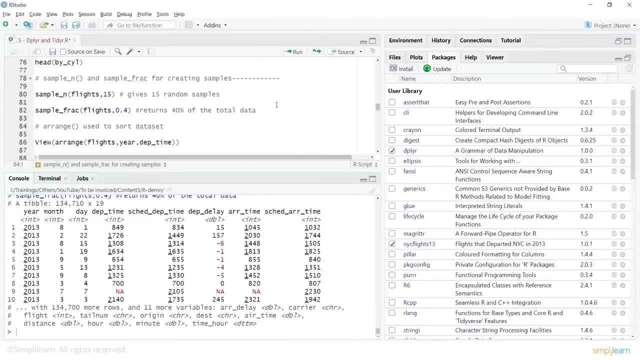 and then you can look at the value of that. now. what we can also do is we can use arrange function. so, like we were doing a grouping by, or we were trying to pull out a particular column, so in the same way we can use arrange, which is a convenient 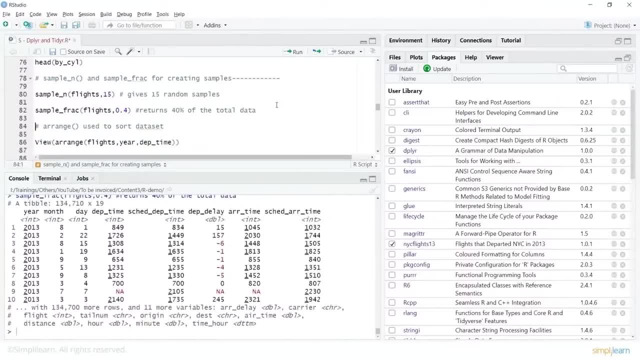 some portion of the data. so you can do this, which is very useful function, and then you can look at the value of that. now, what we can also do is we can use arrange function so like we were doing a grouping by or we were trying to pull out a particular column. 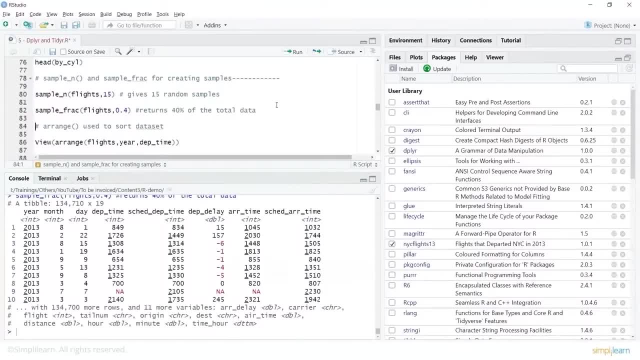 so in the same way we can use arrange, which is a convenient way of sorting than your base R sorting. so for arrange function, let's do a view based on arrange. so we will work on the flights data set which we have, and here what we would want to do is 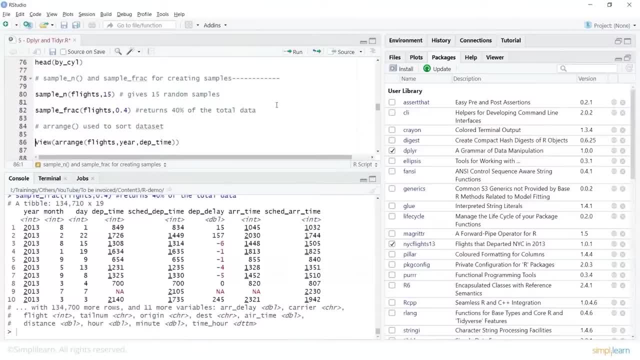 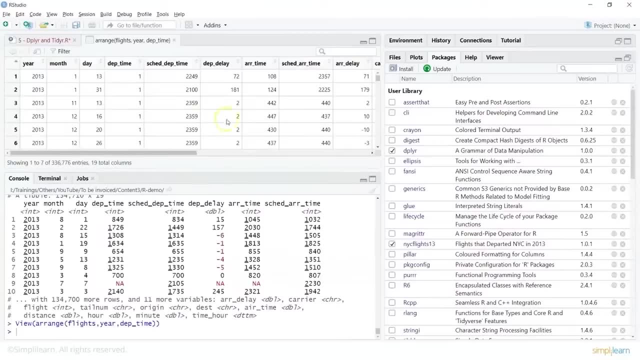 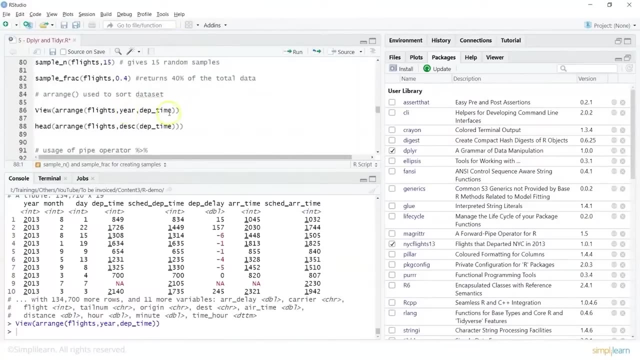 we would want to arrange the flights data set which is based on year and departure time and we are doing a view out of it so that basically gives me the data which is arranged based on your year and departure time. now I can do a head to give me some highlighting of that data. 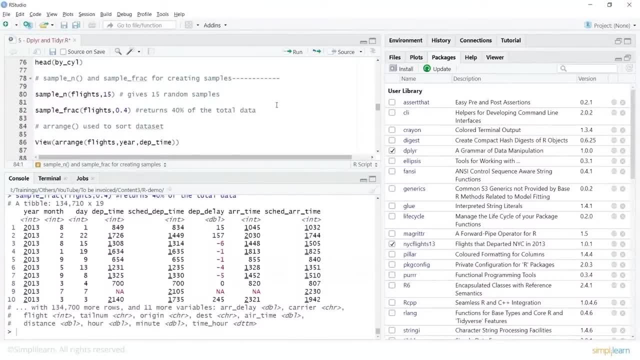 way of sorting than your base R sorting. so for arrange function, lets do a view based on arrange. so we will work on the flights data set which we have and here what we would want to do is we would want to arrange the flights data set which is based. 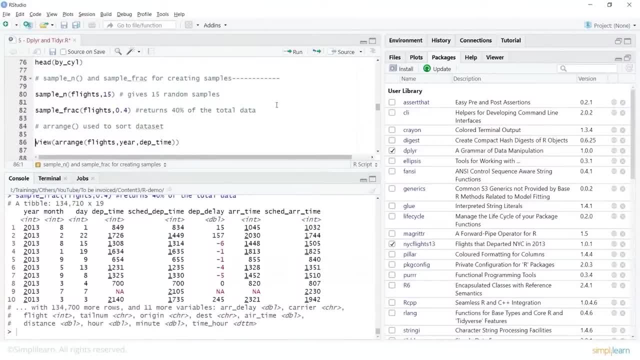 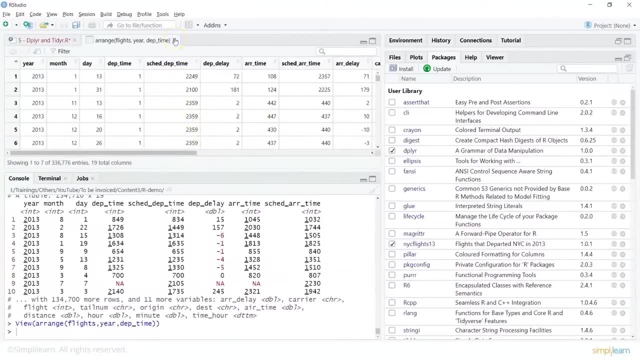 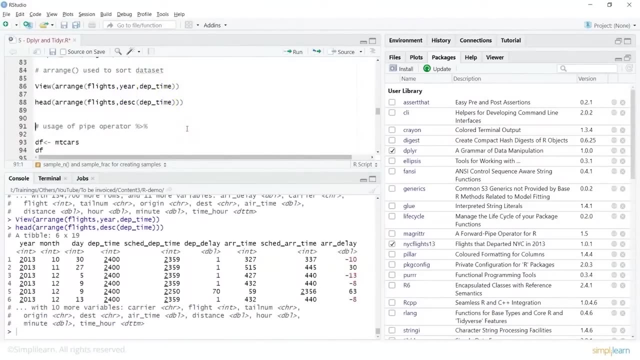 on year and departure time and we are doing a view out of it so that basically gives me the data which is arranged based on your year and departure time. now I can do a head to give me some highlighting of that data. now the piping operator- what we are using- can be used. 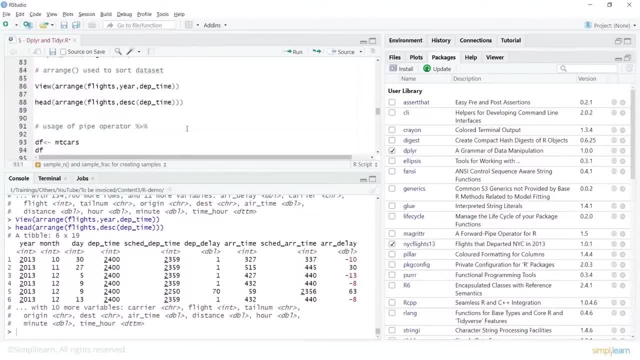 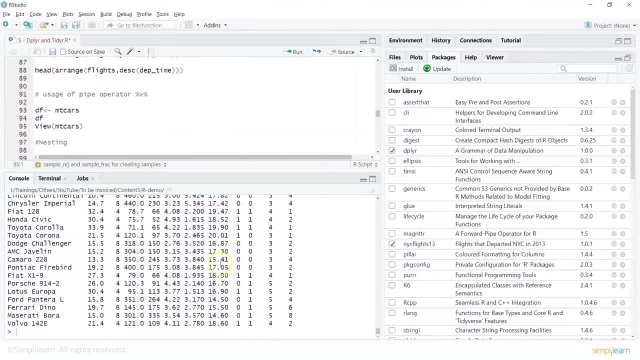 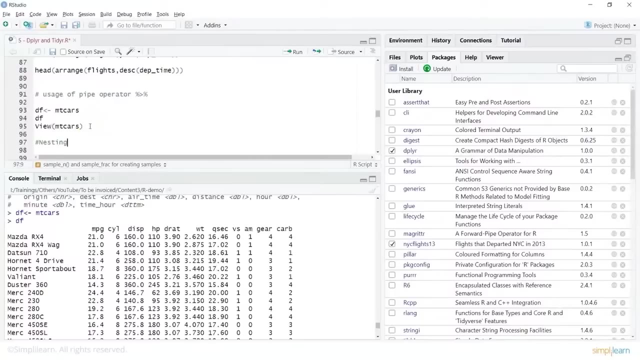 in these ways also. so here I will say DF. I will just assign the data set empty cars to it. lets look at the DF, which has basically your different models. you can obviously look at the head or view of it to look at useful information. we can also go for nesting. 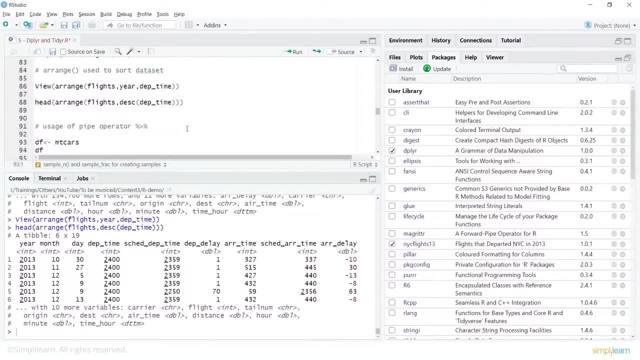 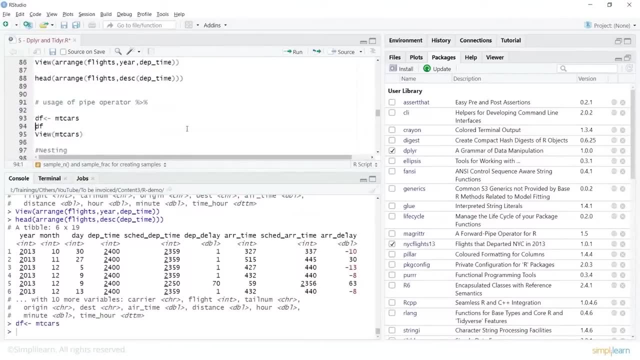 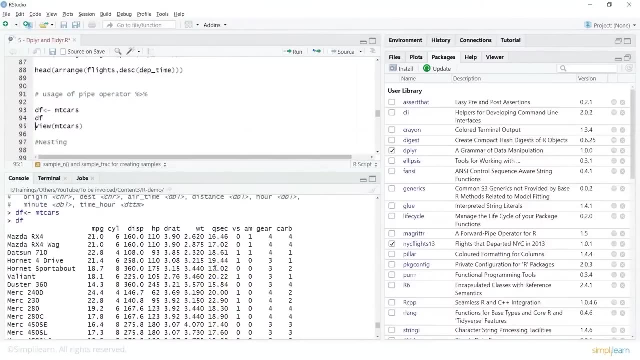 now the piping operator, what we are using, can be used in these ways also. so here I will say df, I will just assign the data set empty cars to it. let's look at the df, which has basically your different models. you can obviously look at the head. 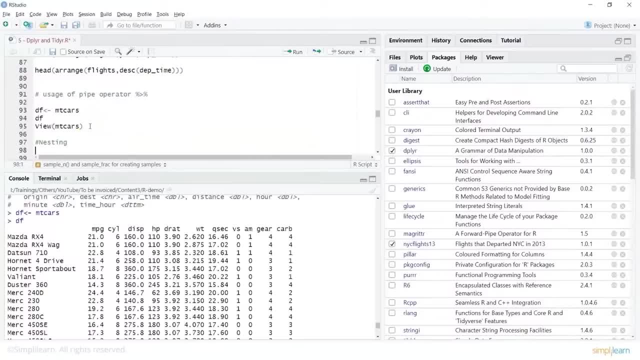 or view of it, to look at useful information. we can also go for nesting options, which can be useful. so we are creating a variable called result here now that has the arrange function. so what does this arrange function do so when we would want to use arrange to sort the data? 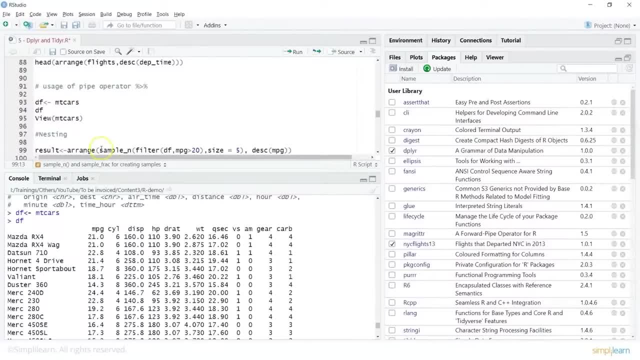 so I would want to sort the data. but what data would I sort? so I will use sample n, which will give me some portion of the data, or some sample data. now, what is that sample data? so here we are using nesting. that is earlier, when we did a sample. 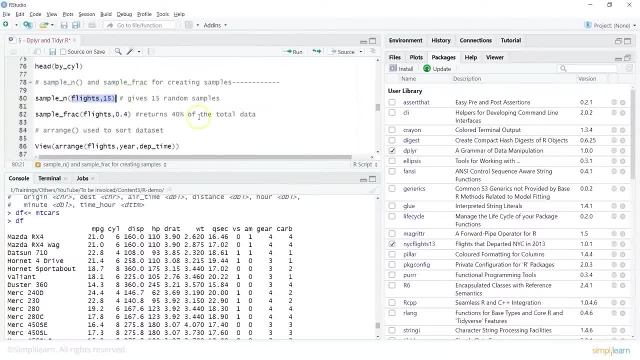 we just said data and how many random samples we want, but instead of giving that, what we are going to do is we are going to use filter here. now. this filter will work on df, so filtering will happen based on the mileage which is greater than 20. 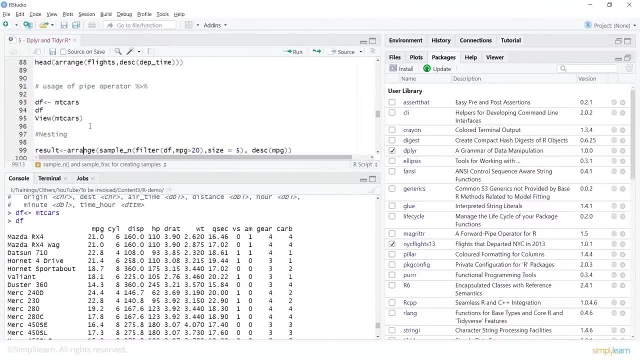 options which can be useful. so we are creating a variable called result here now that has the arrange function. so what does this arrange function do? so when we would want to use arrange to sort the data? so I would want to sort the data, but what data would I sort? so I 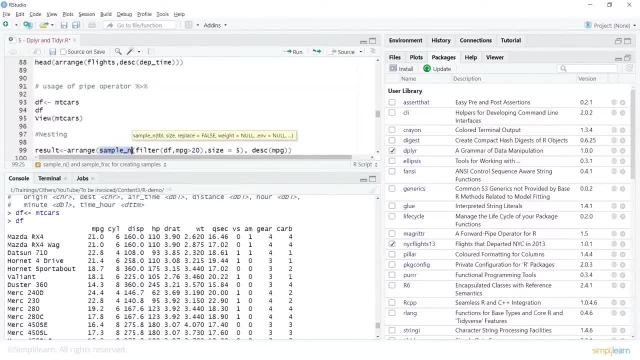 will use sample n, which will give me some portion of the data, or some sample data. now, what is that sample data? so here we are using nesting. that is earlier when we did a sample. we just said data and how many random samples we want, but instead of 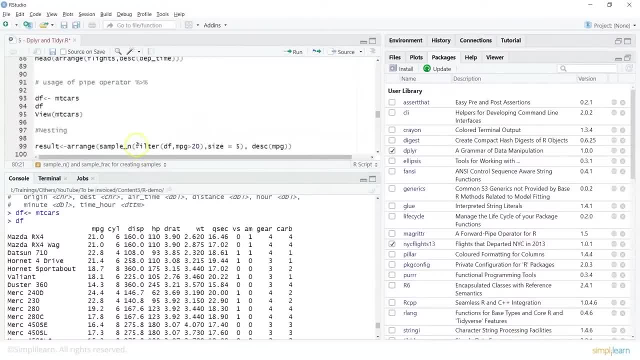 giving that. what we are going to do is we are going to use filter here. now. this filter will work on DF, so filtering will happen based on the mileage which is greater than 20. I will say size is 5 and I would want to basically arrange this in a descending 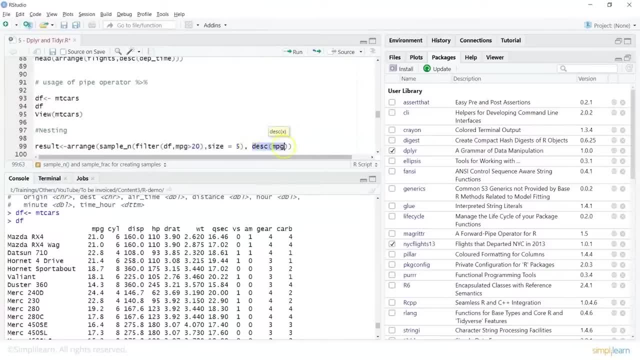 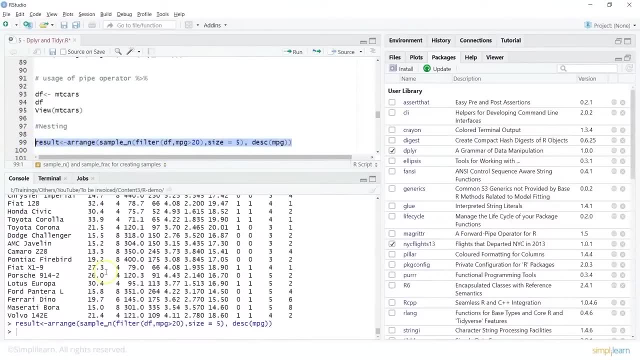 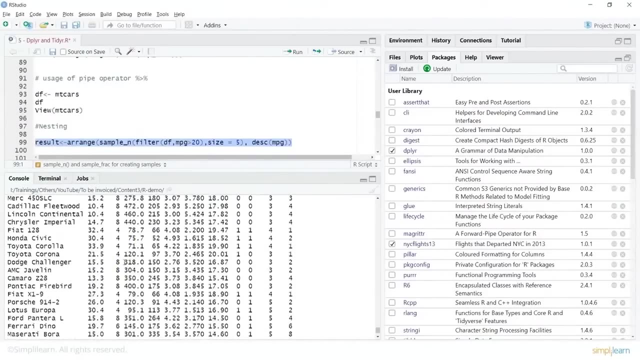 order. so I am using the DES on this particular mileage column. by default, it is always ascending, so lets get the result out of this, which will basically show me the mileage details in a descending order. so this is my data frame and now we can look at the result, what we have. 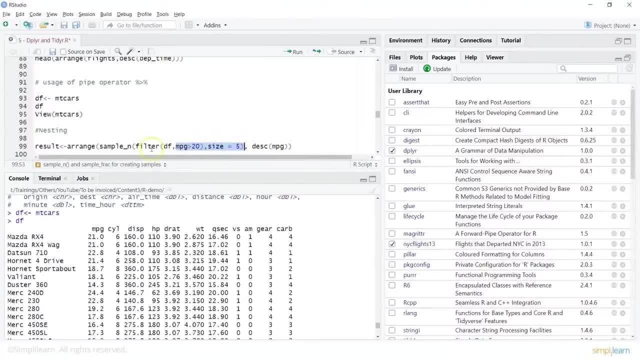 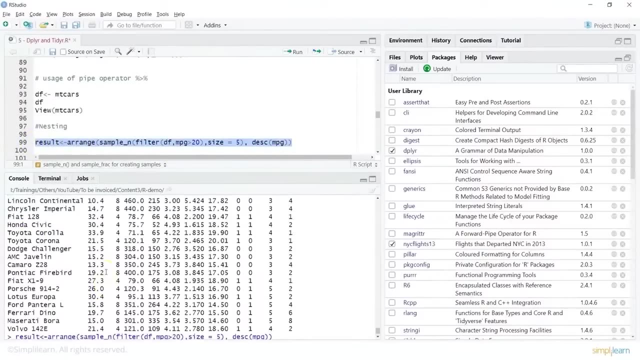 I will say size is 5 and I would want to basically arrange this in a descending order. so I am using the des on this particular mileage column. by default it is always ascending, so let's get the result out of this, which will basically show me the mileage details in a descending order. 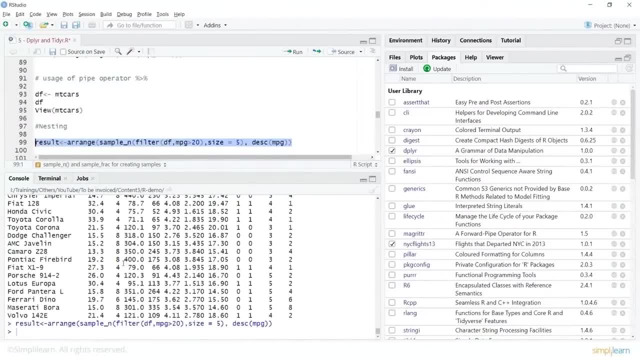 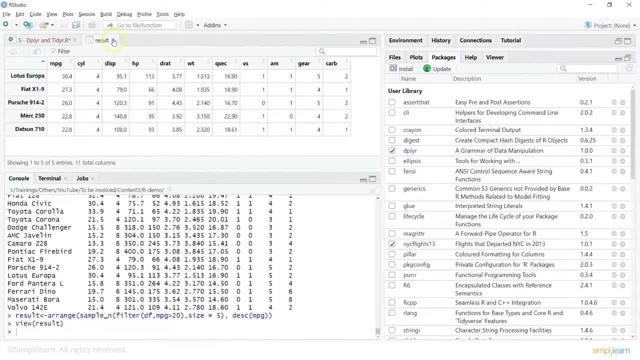 so this is my data frame and now we can look at the result, what we have created. so just do a view or do a head and look at the view. so here you see, mileage, where the highest value is on the top, and we were only interested in 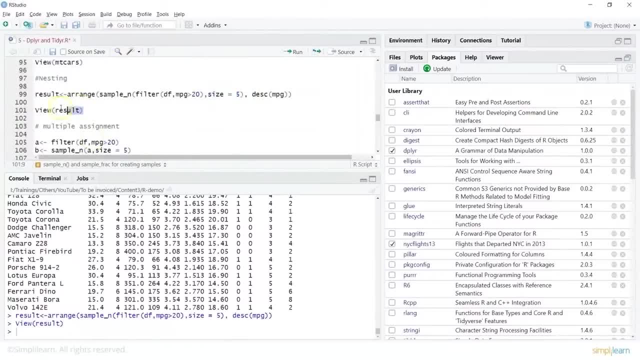 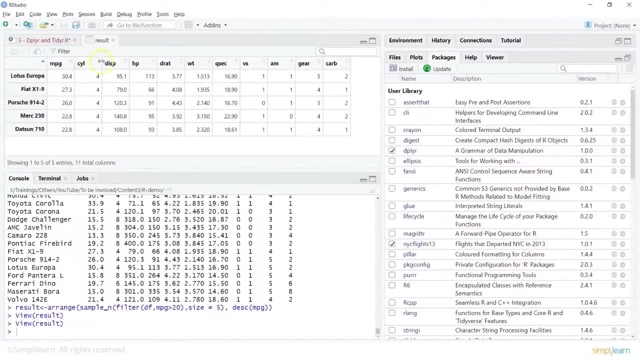 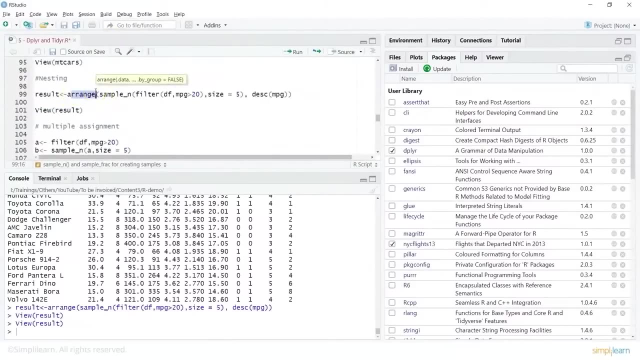 5 values in a random sample. so that's why when you did a view, it shows your 5 values and it shows in a descending order based on mileage. so we have not only used an inbuilt function, we have not only arranged the data, that is, we have sorted the data. 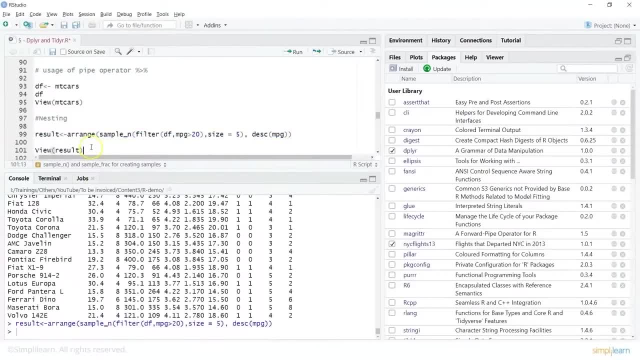 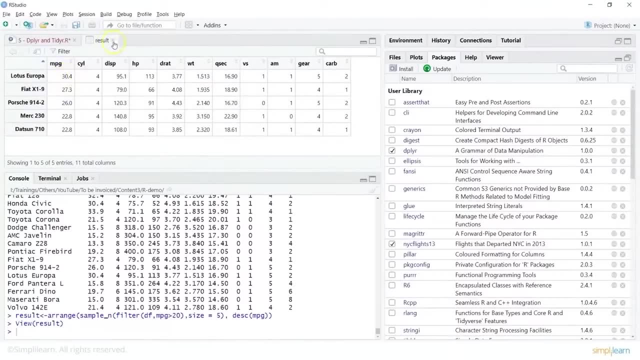 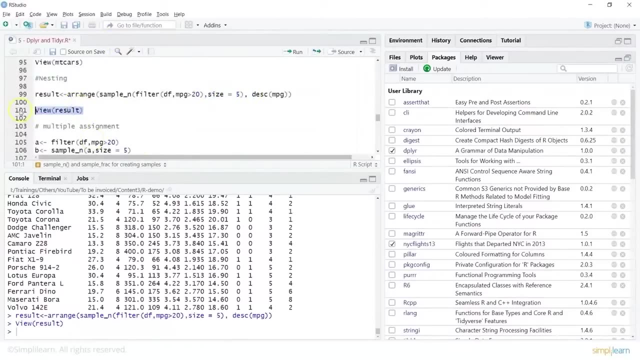 created. so just do a view, or do a head and look at the view. so here you see mileage, where the highest value is on the top, and we were only interested in 5 values in a random sample. so that's why when you did a view, it shows your 5. 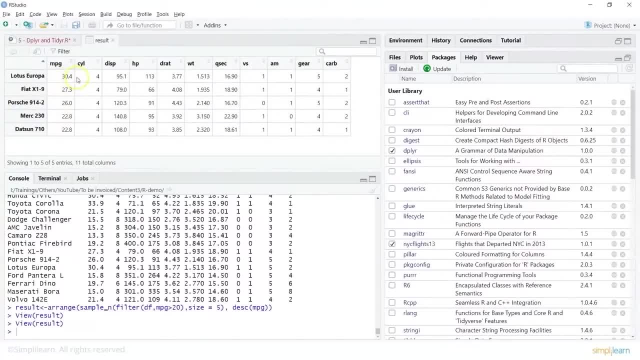 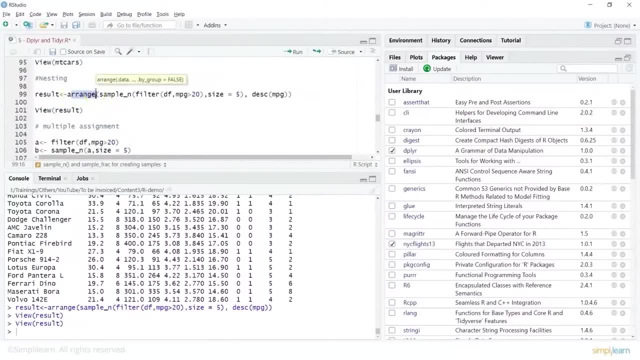 values and it shows in a descending order based on mileage. so we have not only used an inbuilt function, we have not only arranged the data, that is, we have sorted the data, but we have sorted the data based on a descending order. on a particular column, we have 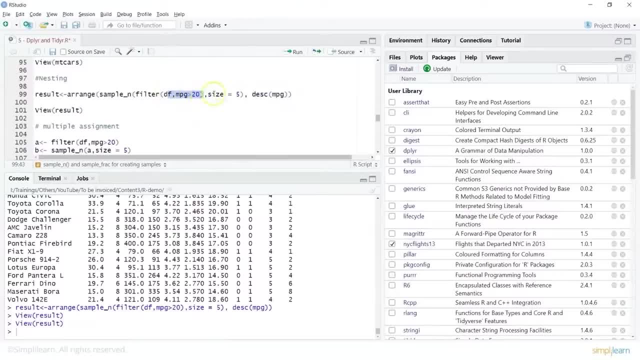 said the value should be greater than 20, and we have also said we just need 5 random samples. now lets look at some other examples. so you can always do a multi assignment, so I can say filter, wherein I am going to use df, which was assigned empty cars, I am. 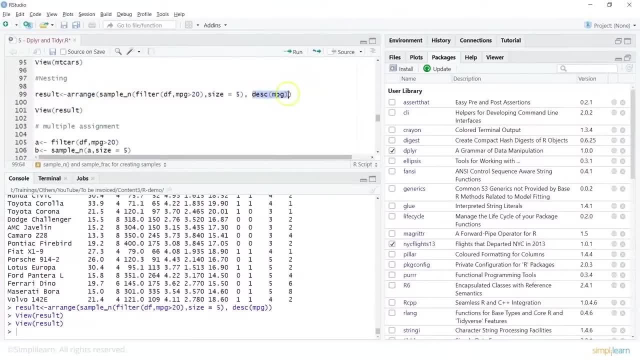 but we have sorted the data based on a descending order. in a particular column, we have said the value should be greater than 20 and we have also said we just need 5 random samples. now let's look at some other examples. so you can always do a multi assignment. 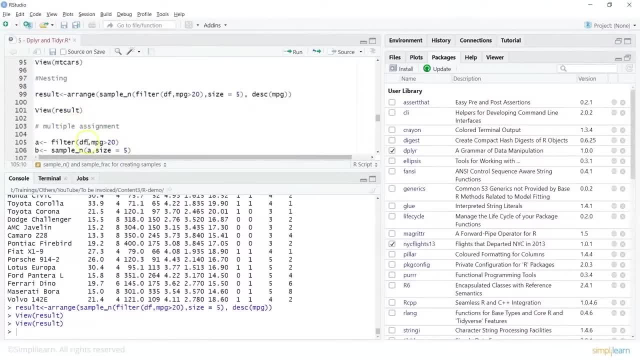 so I can say filter, wherein I am going to use df, which was assigned empty cars. I am going to say: mileage should be greater than 20, then I say b, which is going to get a sample out of a, and I just want 5 random values. 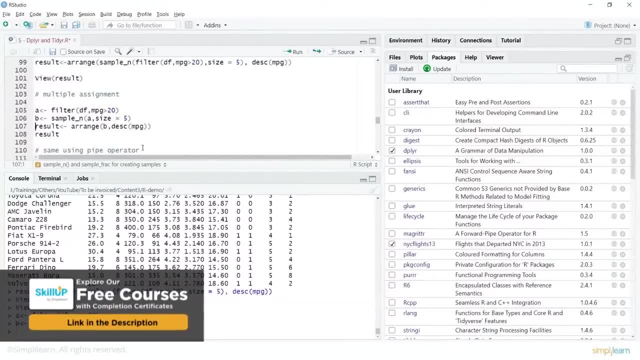 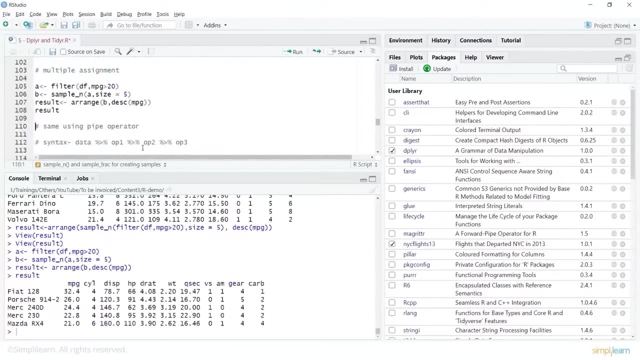 so let's look at that. so we have b, which is going to get a set of 5 values from a. now I will create a result variable which will arrange b, which is sample data, in a descending order. now let's look at the result of this. 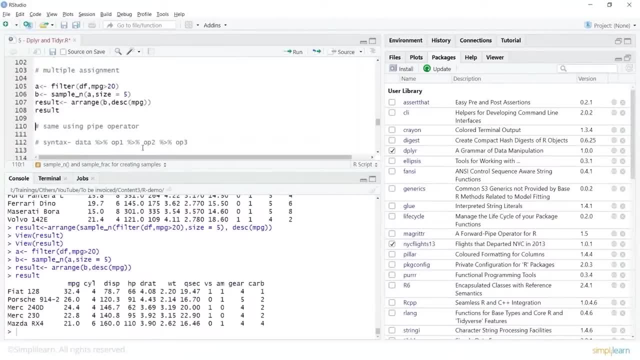 and that basically shows me what we were seeing earlier. so you can do a multi assignment where you can create a variable, get a sample out of it and then basically, whatever is that result, you can arrange that or sort that in a descending or, by default, descending order. 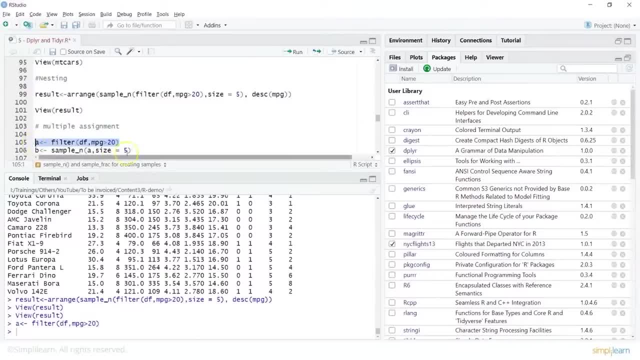 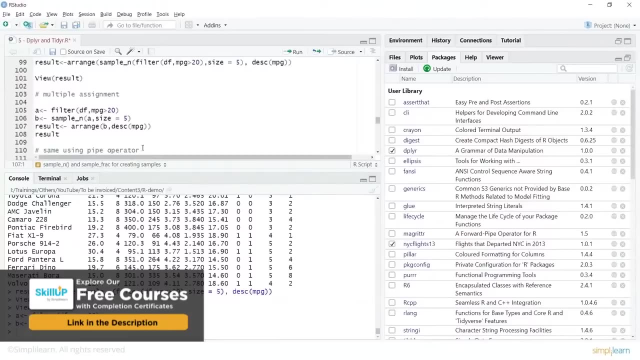 going to say mileage should be greater than 20. then I say b, which is going to get a sample out of a, and I just want 5 random values. so lets look at that. so we have b, which is going to get a set of 5 values. 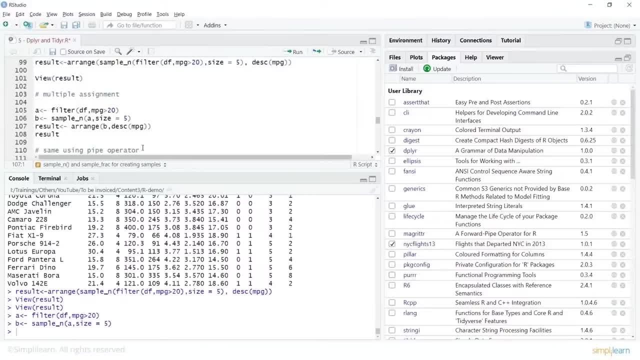 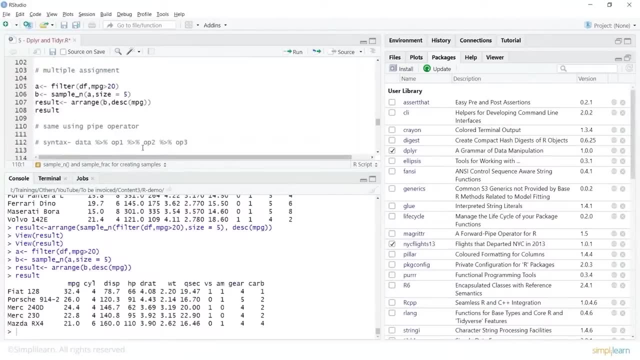 from a. now I will create a result variable which will arrange b, which is sample data, in a descending order. now lets look at the result of this, and that basically shows me what we were seeing earlier. so you can do a multi assignment where you can create a variable. 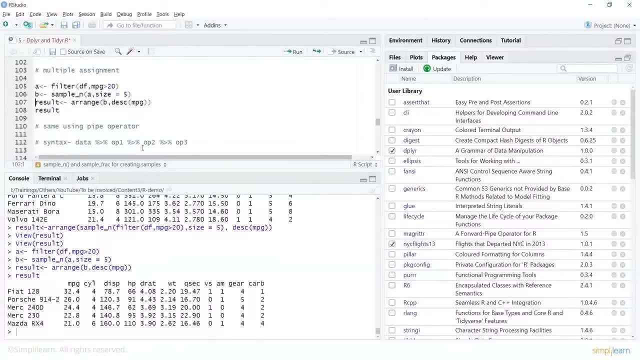 get a sample out of it and then basically, whatever is that result, you can arrange that or sort that in a descending order. by default descending order, so same thing. we can do it using pipe operator, so piping. so here I will say result. I am passing in my df. that is the. 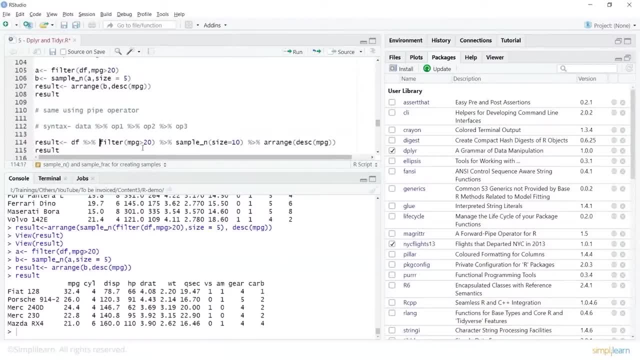 data set I am using piping and which basically tells what you need to do on this particular data set. so I am going to filter out the data based on mileage 50- sorry, mileage 20. then I am going to push that or forward it to get the. 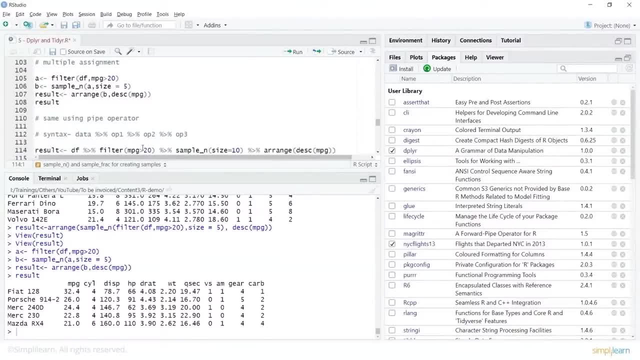 so same thing. we can do it using pipe operator, so piping. so here I will say result. I am passing in my df that's the data set I am using- piping- and which basically tells what you need to do on this particular data set. so I am going to filter out. 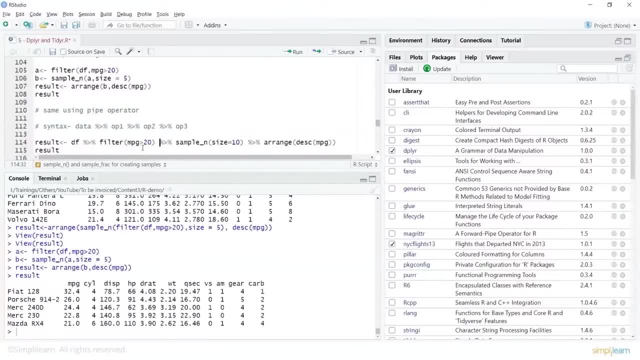 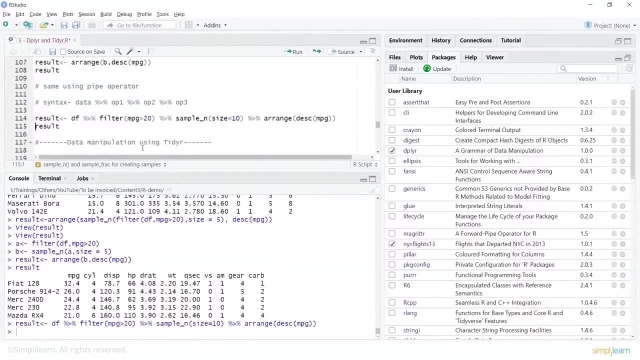 the data based on mileage 50- sorry, mileage 20- then I am going to push that or forward it to get the random sample. and whatever is this random sample is going to be pushed. so you are arranging this in a descending order, so this is one more way of doing it. 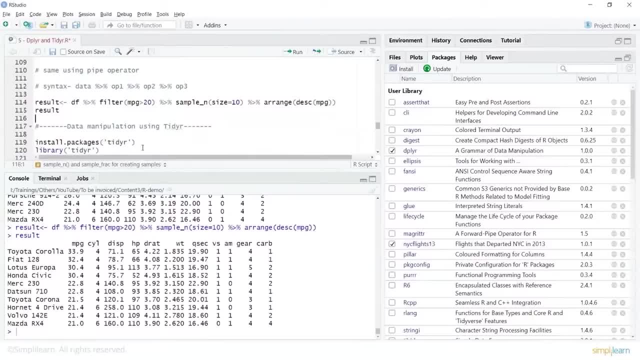 and then, basically, you can look at the result. so these are some simple examples where you can use your dplyr with multiple assignments or using your nesting to filter out the data. you can also do a arrange, which is to sort the data. you can get some random samples out of it. 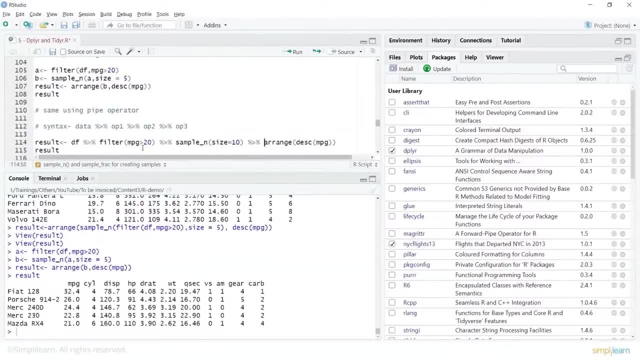 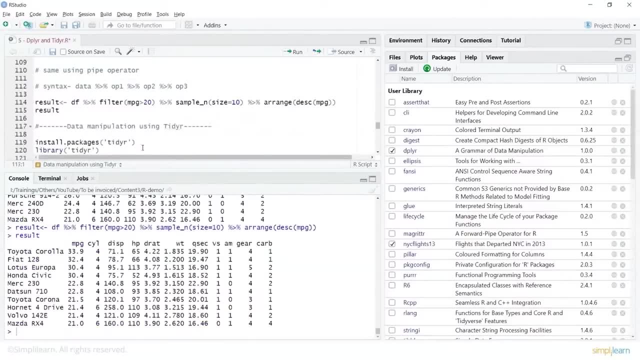 random sample, and whatever is this random sample is going to be pushed. so you are arranging this in a descending order, so this is one more way of doing it and then, basically, you can look at the result. so these are some simple examples where you can use your dplyr with multiple. 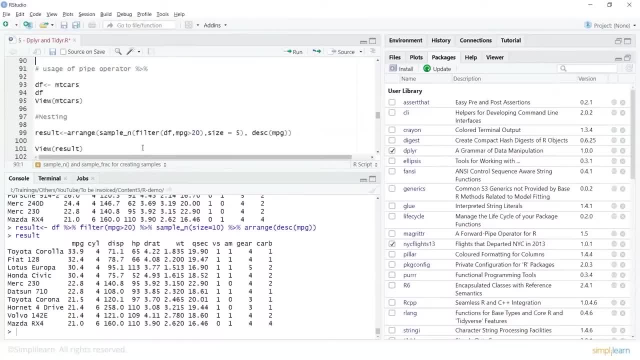 assignments or using your nesting to filter out the data. you can also do a arrange, which is to sort the data. you can get some random samples out of it. you can summarize the data. you can also summarize the data based on one or two or multiple columns and you can use some inbuilt. 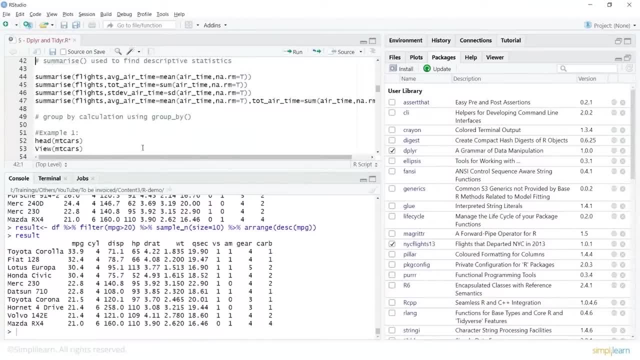 functions. to summarize the data based on some functions which are applied on the variables or on the columns, you can transmute it. where you would be interested in only looking at one column, you can mutate it. where you want to add a new column, you can slice it. 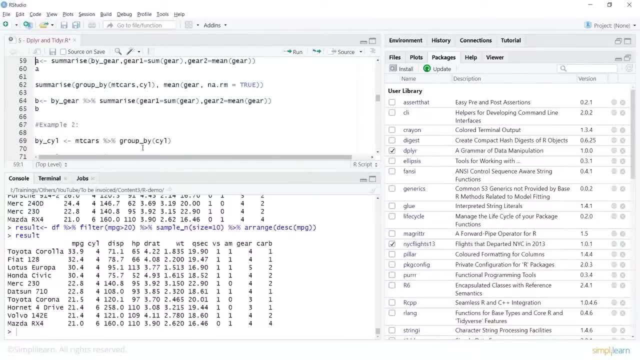 you can summarize the data. you can also summarize the data based on one or two or multiple columns and you can use some inbuilt functions to summarize the data based on some functions which are applied on the variables or on the columns. you can transmute it where you would be interested in. 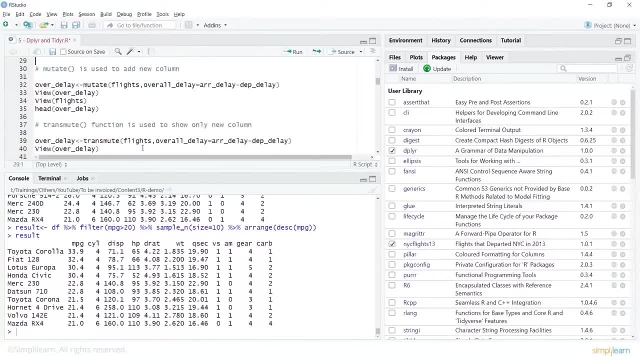 only looking at one column. you can mutate it. where you want to add a new column, you can slice it and you can give the conditions where you can say and or or to filter out the data. so what we can also do is on this particular data set. 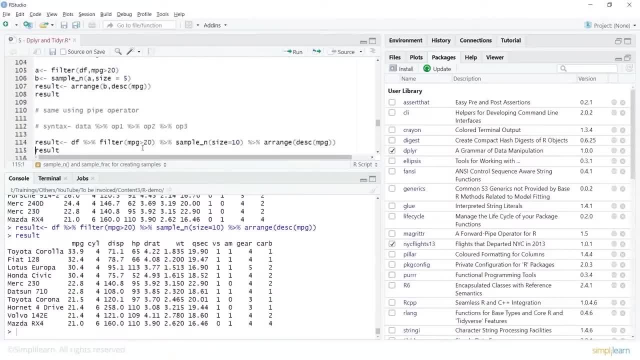 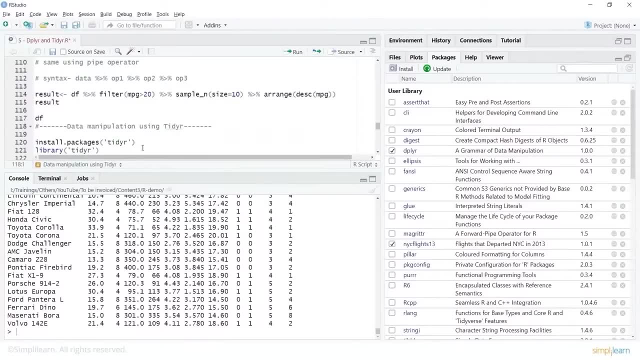 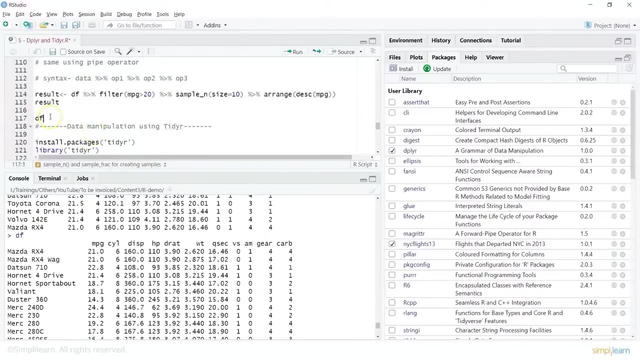 which we have say, for example, df, where I have my data. let's look at this one, and if I just do a df at this point, it shows me my data set. and if you would be interested only in particular columns, then your dplyr also allows you to. 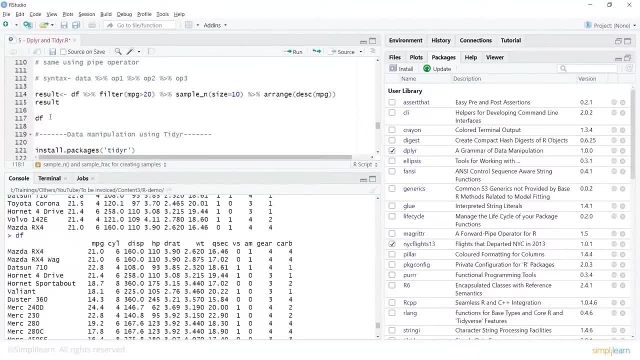 either we can do a filter or we can simply do a select. now for selecting, we can choose our data. so for example, I will say: df underscore. I am interested in mileage, I am interested in horse power. might be, I am interested in your cylinders in this and for this one. 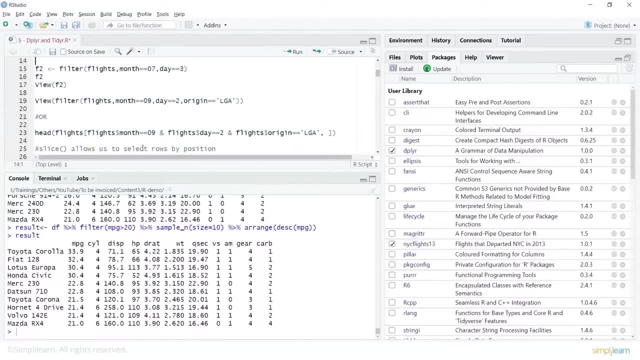 and you can give the conditions where you can say and or to filter out the data. so what we can also do is, on this particular data set which we have, say, for example, df, where i have my data, let's look at this one. and if i just do a, 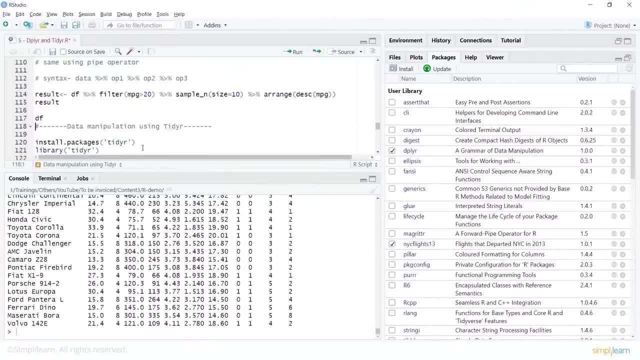 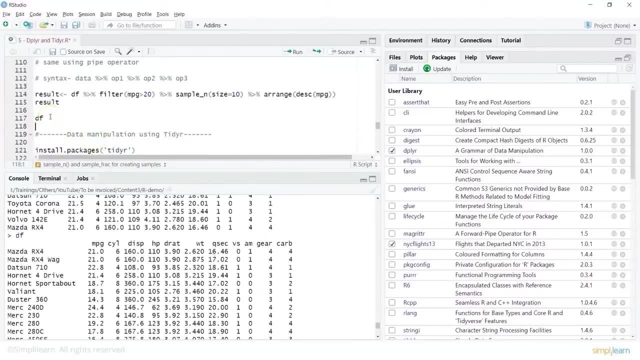 df at this point it shows me my data set, and if you would be interested only in particular column, then your dplyr also allows you to. either we can do a filter or we can simply do a select. now for selecting, we can choose our data. so, for example, i'll say: 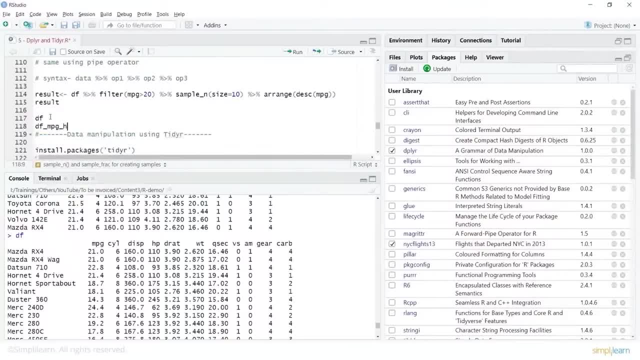 df underscore. i'm interested in mileage. i'm interested in horsepower, might be, i'm interested in your cylinders. in this and for this one, what i can do is when i would want to do a select, i can basically say: selected df, let's call it some name. 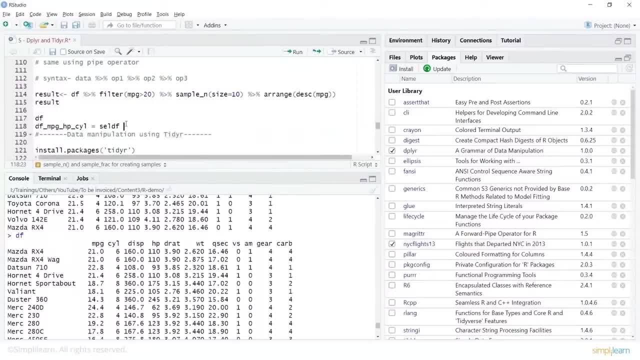 i can say control, shift m, which is for piping, and then basically what you can do is you can do a select and you can choose your columns. so i was interested in mileage, i was interested in horsepower, i was interested in cylinder, and here what i'm doing is i'm using a 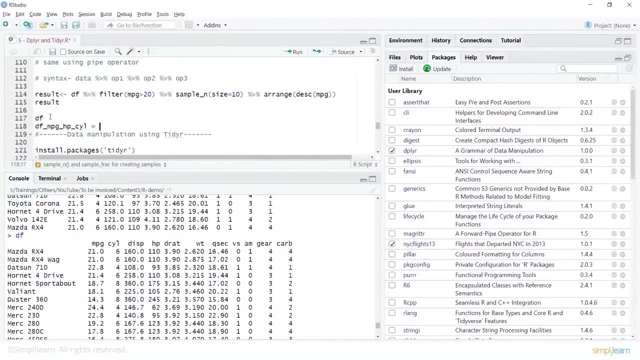 what I can do is select. I can basically say selected df, let's call it some name. I can say control shift m, which is for piping, and then basically what you can do is you can do a select and you can choose your columns. so I was interested in mileage. 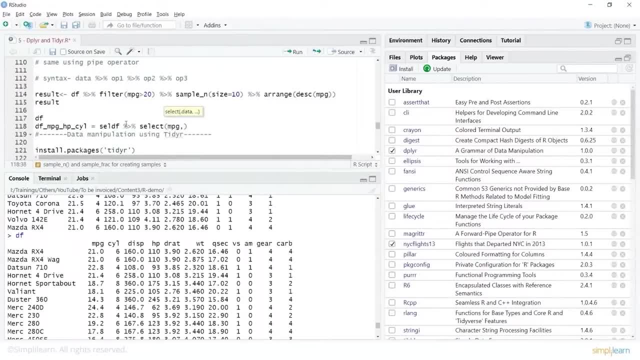 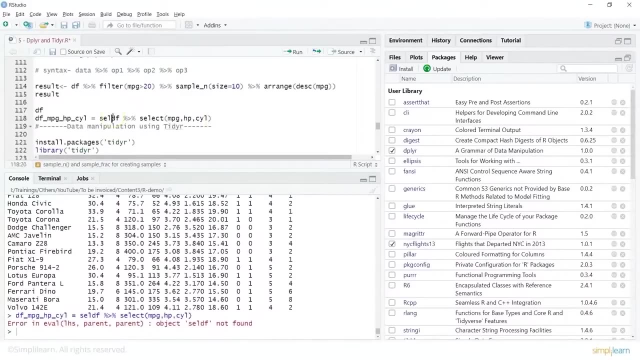 I was interested in horse power, I was interested in cylinder, and here what I am doing is I am using a select where I can look at the new data frame. so let's do this, and I am sorry, here we will have to give it df. this is where. 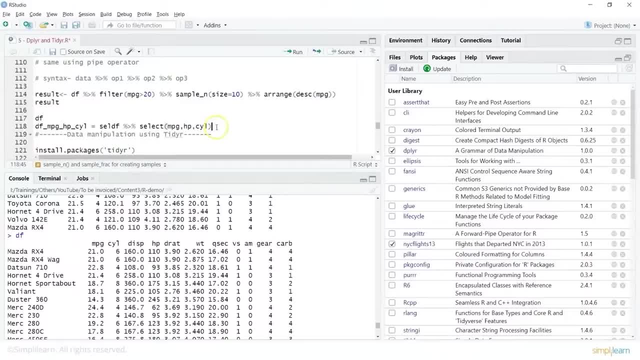 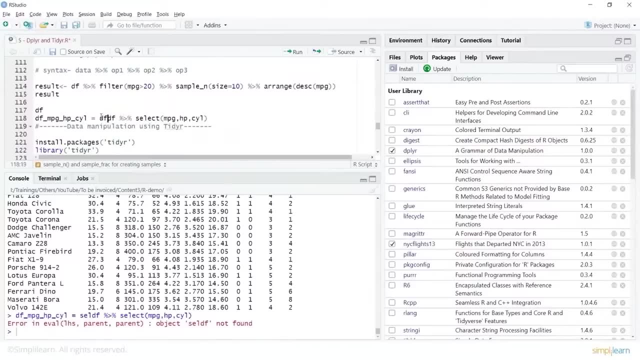 select where i can look at the new data frame. so let's do this, and i'm sorry, here we will have to give it df. this is where you are passing in your data. yeah, now this one is done and we can look at the value of this one by just doing a. 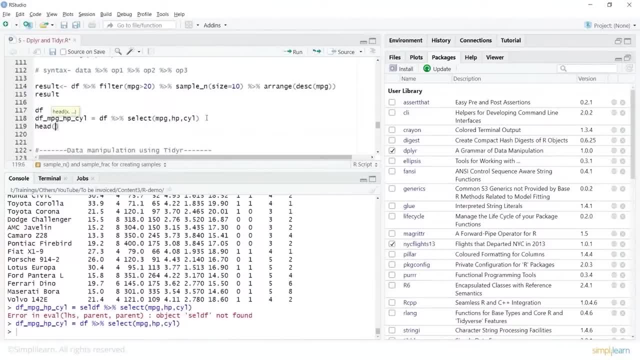 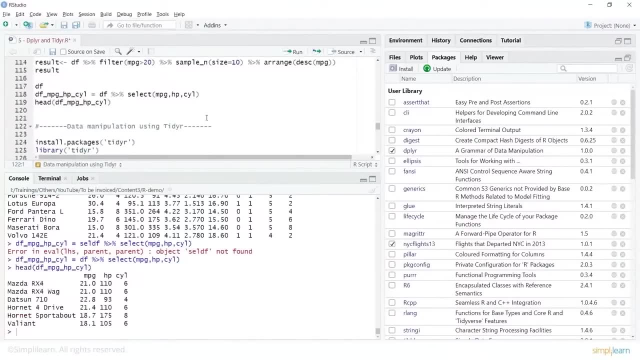 df or head on df, underscore mileage, horsepower, cylinder and look at the selected result so you can be looking at selective columns. i could have done this filter, but filter will always look for a condition, say your mileage is greater than 20, or might be your cylinders are more than 4. 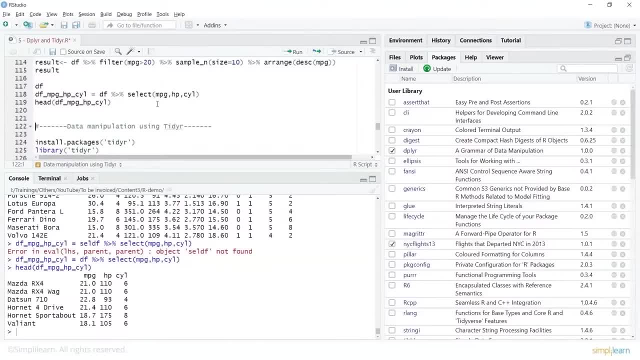 or something else, but when you do a select you are selecting specific columns. so view always gives you all the columns, head gives you highlight, but then select can be useful when we are interested in looking at only specific data. so this is how you can use deep layer for 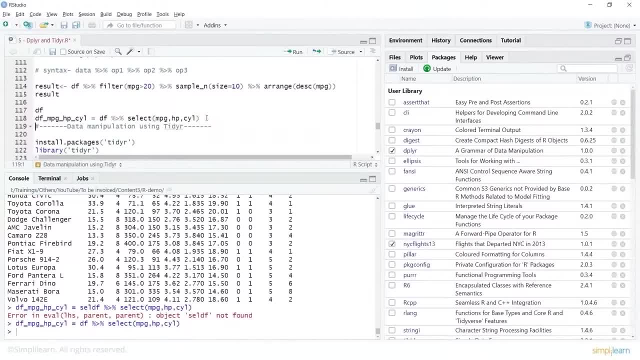 you are passing in your data. yeah, now this one is done and we can look at the value of this one by just doing a df or head on df, underscore, mileage or power cylinder and look at the selected result. so you can be looking at selective columns. I could have done this filter. 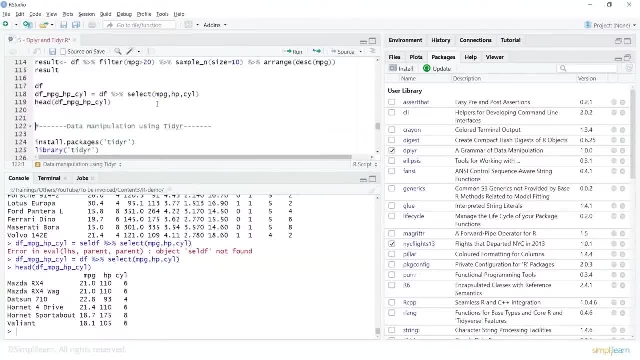 but filter will always look for a condition, say your mileage is greater than 20, or might be your cylinders are more than 4 or something else. but when you do a select, you are selecting specific columns. so view always gives you all the columns, head gives you highlight, but then 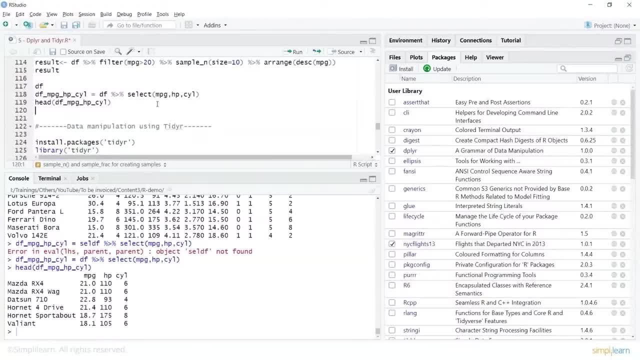 select can be useful when we are interested in looking at only specific data. so this is how you can use dplyr for manipulation, for your data transformation, for basically filtering out the data by selecting particular data and then working on it. so, similarly, there is one more package. 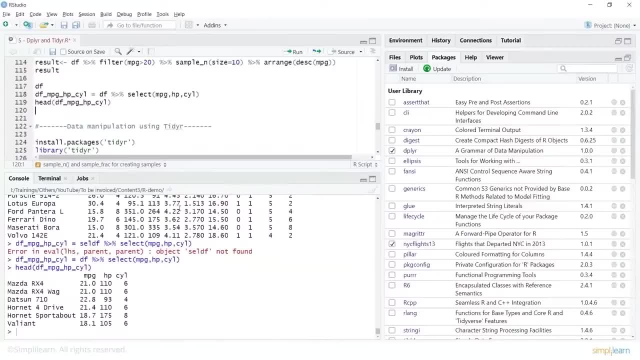 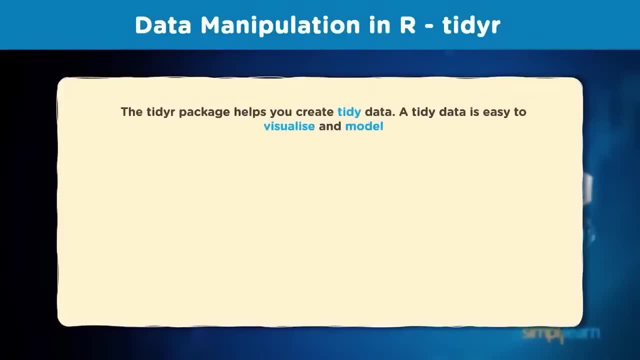 called tidr, and we will see how we can use data manipulation done using your tidr package. let's learn about the tidr package. it makes it easy to tidy your data and this basically helps you creating a more cleaner data so which is easy to visualize and model. 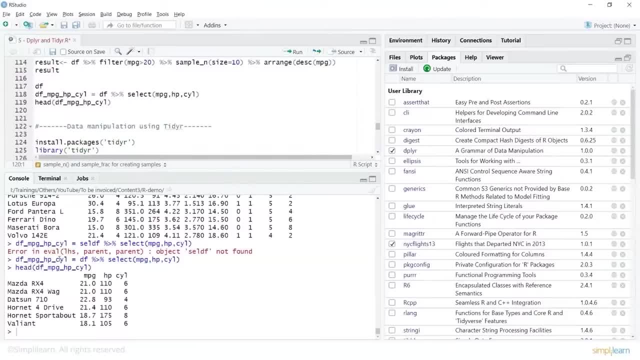 manipulation for your data transformation, for basically filtering out the data by selecting particular data and then working on it. so, similarly, there is one more package called tidy r and we'll see how we can use data manipulation done using your tidy r package. let's learn about the tidy r package. 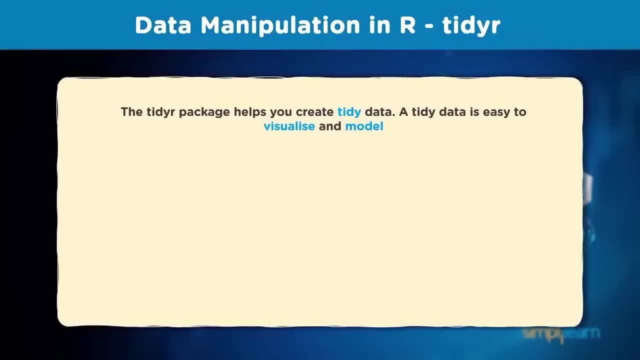 it makes it easy to tidy your data and this basically helps you creating a more cleaner data, so which is easy to visualize and model. now this comes with mainly four functions. so you have gather which makes your data wide or it makes wide data longer, so that is basically used to stack. 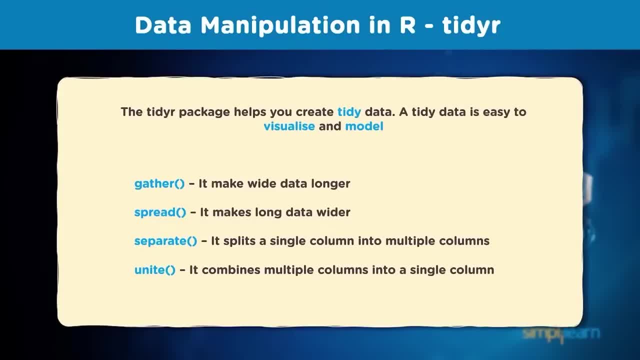 up multiple columns. you have spread function which makes long data wider. that is, stacking the data together, or stack, if you would want to unstack the data to data and you are talking about data which has same attributes, and then your spread can spread the data across multiple. 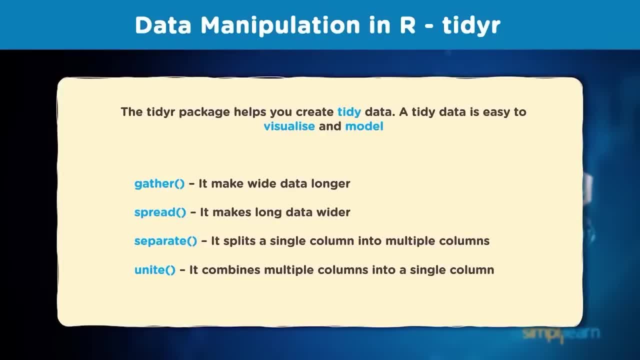 columns. you have separate, which is function which splits single column into multiple columns, and to complement that you have one more function which is unite and that combines multiple columns into single columns. so these are four main functions which are used in your tidy r package. so let's 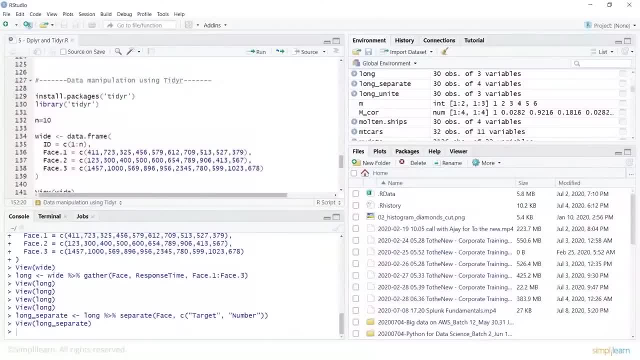 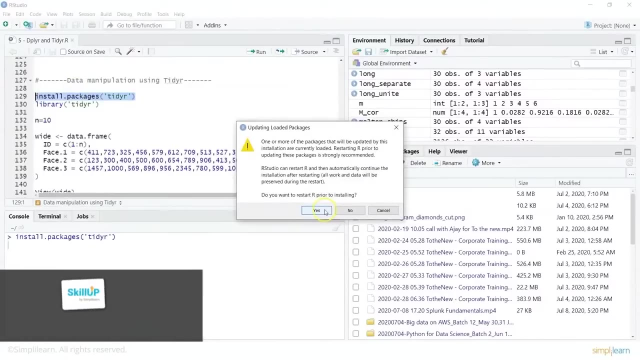 look how we work with this. so let me bring up my r studio here now for this. first is let me just clean up my screen here doing a control l, so i will install the package. it is already installed, but we can just do a control enter and then. 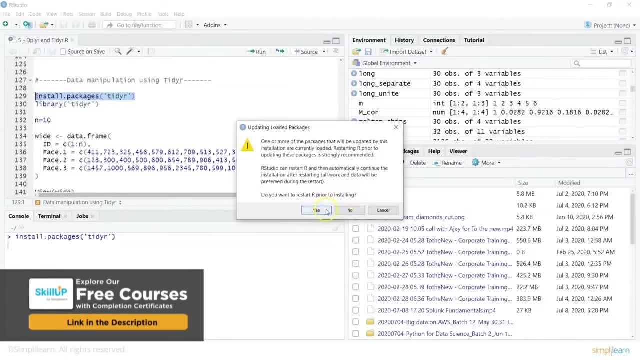 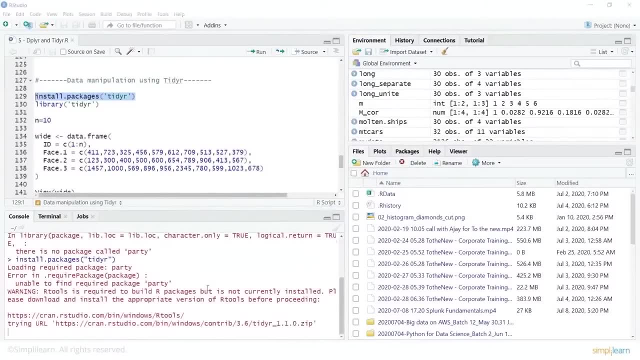 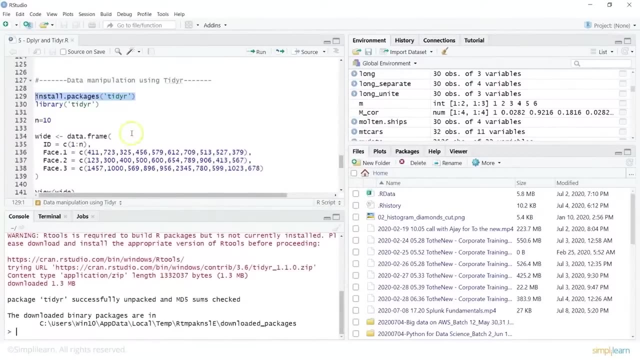 i can say: do you want to restart r prior to reinstall? to install. i will say ok and it is basically going to get the package. now it says: package tidyr. that is, tidyr has been successfully unpacked. let's use that package using our library function and 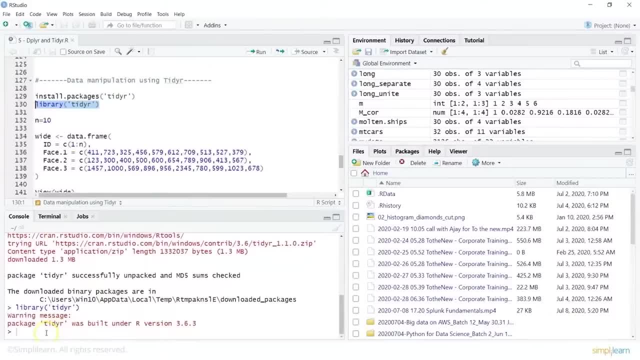 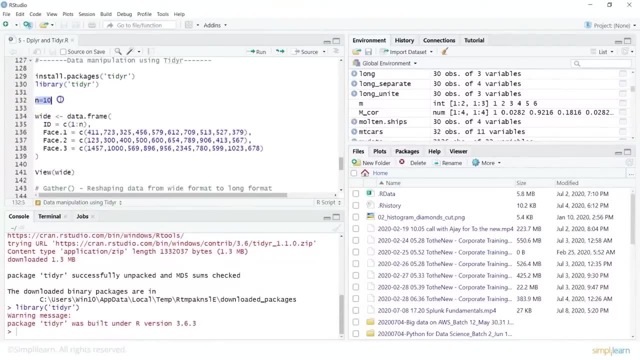 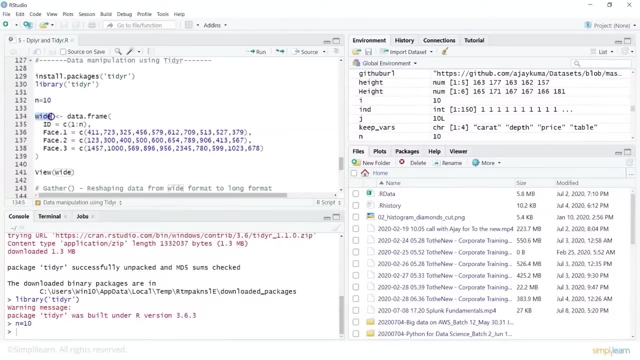 that was build under r version 3.6. now i can basically start using these functions. so, for example, here we are creating a data frame. so let's say n is 10, and then we basically would say we will call it white. now, that's the. 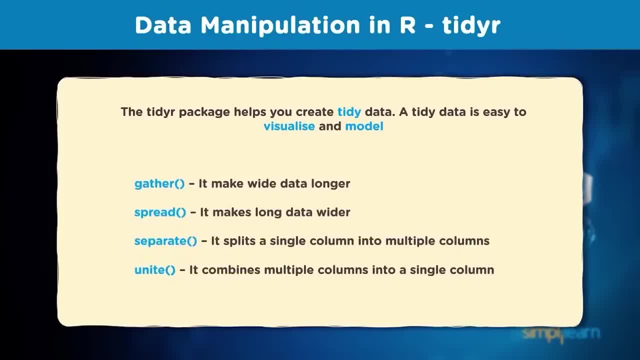 now this comes with mainly four functions. so you have gather, which makes your data wide, or it makes wide data longer, so that is basically used to stack up multiple columns. you have spread function, which makes long data wider. that is, stacking the data together, or stack if you would want to. 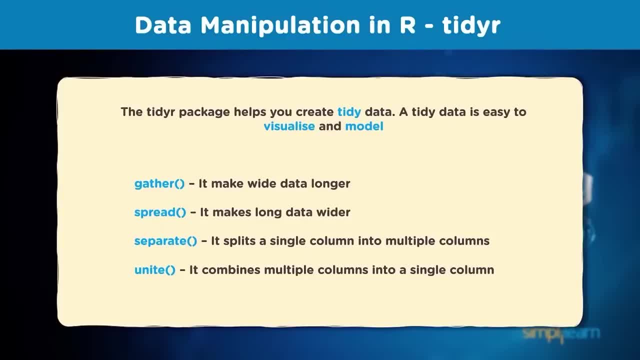 unstack the data to data and you are talking about data which has same attributes, and then your spread can spread the data across multiple columns. you have separate, which is function which splits single column into multiple columns, and to complement that you have one more function which is unite. 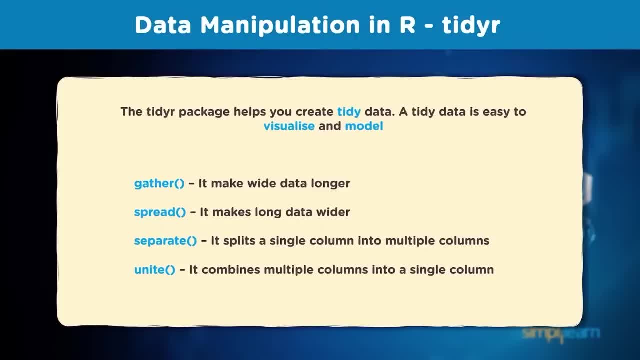 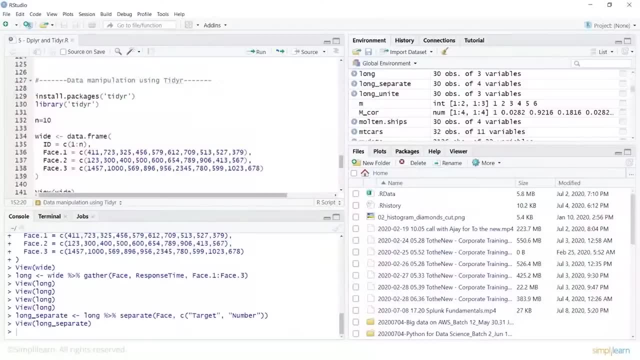 and that combines multiple columns into single columns. so these are four main functions which are used in your tidr package. so let's look how we work with this. so let me bring up my R studio here now, for this first is: let me just clean up my 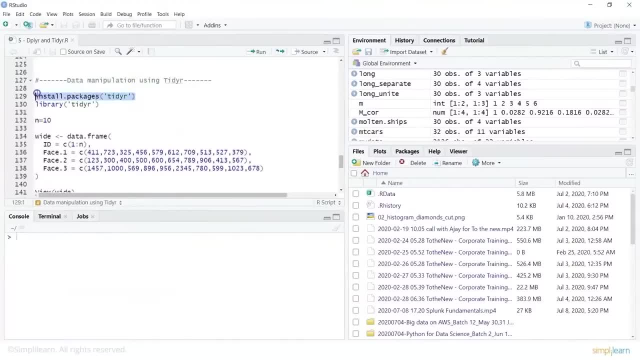 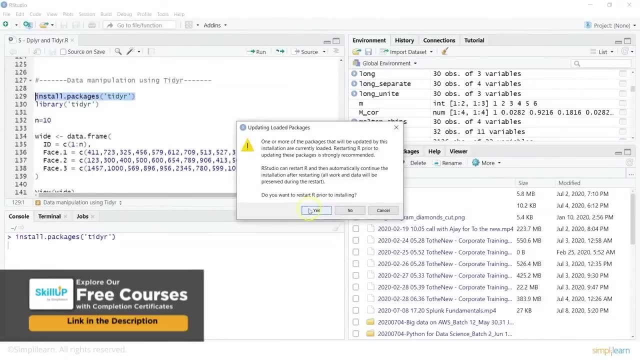 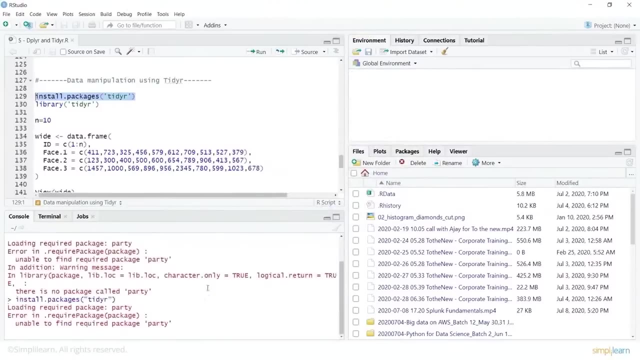 screen here doing a control L, so I will install the package. it is already installed, but we can just do a control enter and then I can say: do you want to restart R prior to reinstall. I will say okay and it is basically going to get the package. 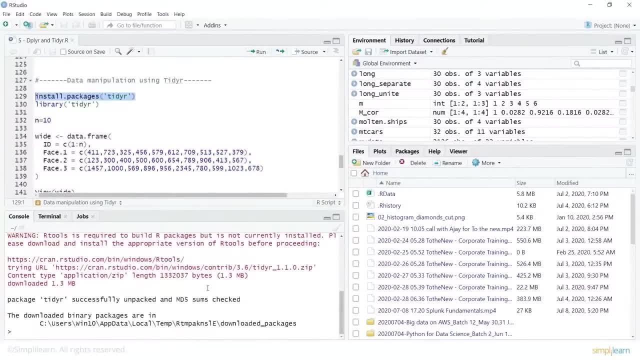 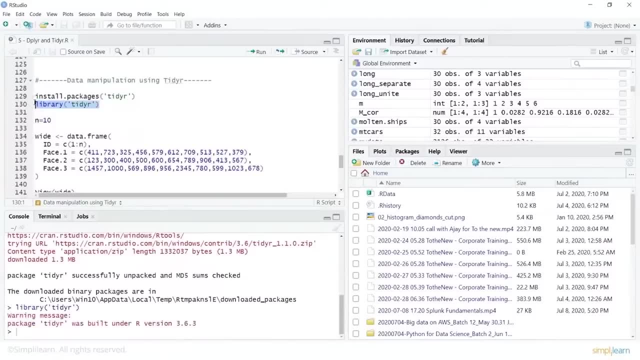 now it says: package tidyr. that is, tidyr has been successfully unpacked. let's use that package using our library function, and that was build under R version 3.6. now I can basically start using these functions. so, for example, here we are creating a data frame. 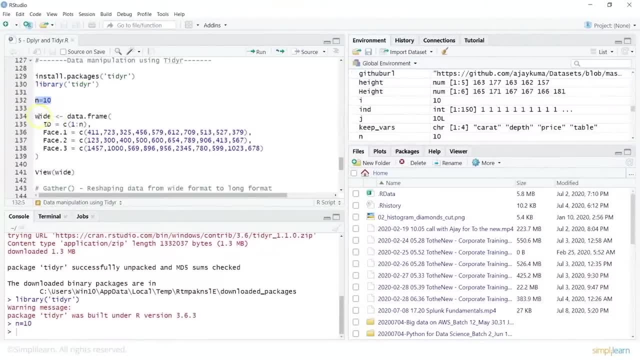 so let's say n is 10 and then we basically would say we will call it wide. now that is the variable name. I am using the data dot frame function. I am saying id, which will be 1 to n, so that will take the values from. 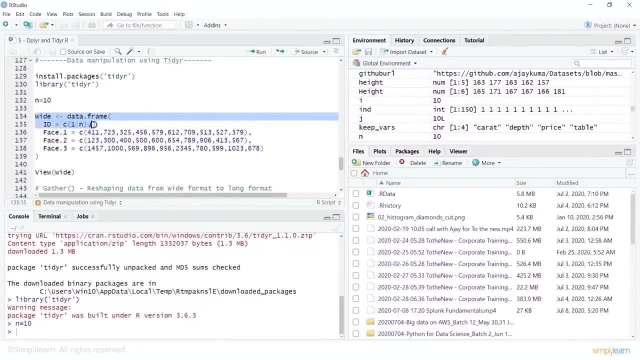 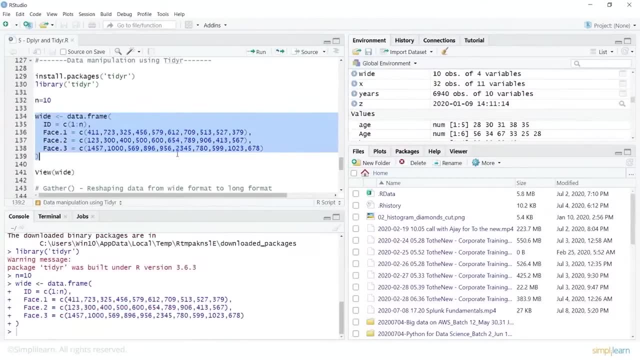 1 to 10, and then these are the values which have 10 entries. so this is a vector: phase 1, phase 2, phase 3: let's create a data frame out of it. now that is done, we can have a look at our data frame. 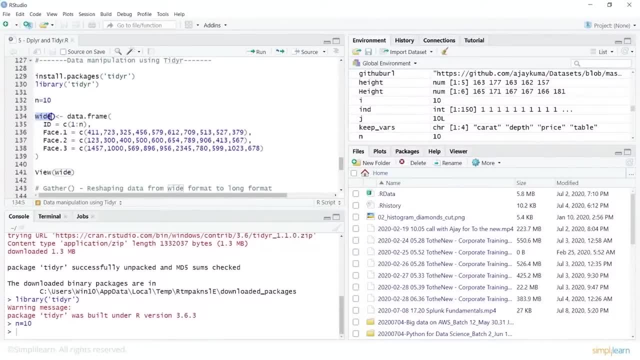 variable name. i am using the data dot frame function. i am saying id, which will be 1 to n, so that will take the values from 1 to 10, and then these are the values which have 10 entries. so this is a vector. face 1, face 2, face 3: let's create. 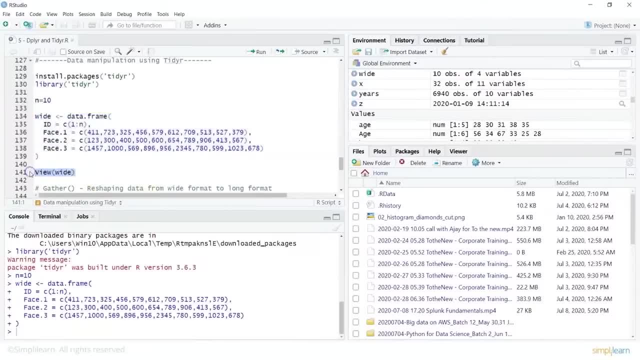 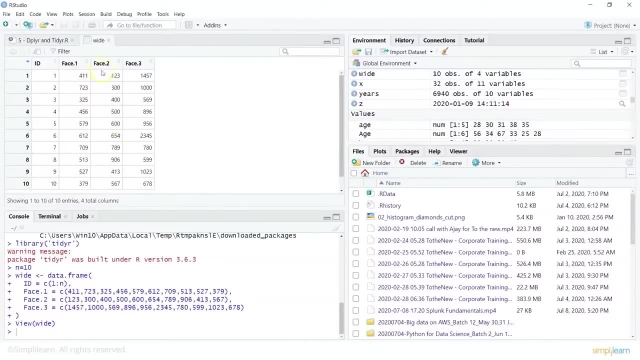 a data frame out of it. now that's done, we can have a look at our data frame by just doing a view wide and that shows me the id column and it has face dot 1, face dot 2 and face dot 3. now we can use our. 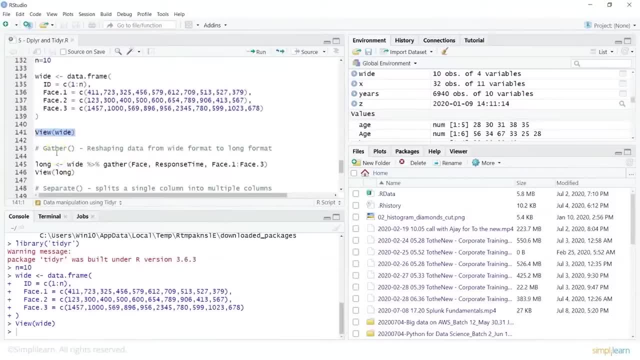 function. so, for example, we can work with gather, that is, reshaping the data from wide format to long format, and basically you can say stacking up multiple columns. so let's see how we do that here. i will call it long. i am working on wide, i am. 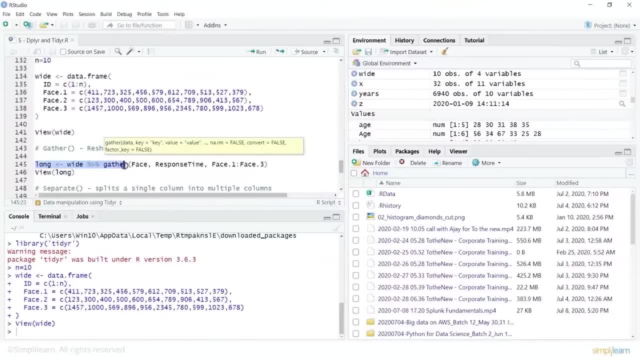 using the piping functionality, and then i am using gather. so this one, i will say what will be the data which i will use. so we are using wide as a data frame. then i am saying response time, so that will be basically one more column and then you have your columns which you would 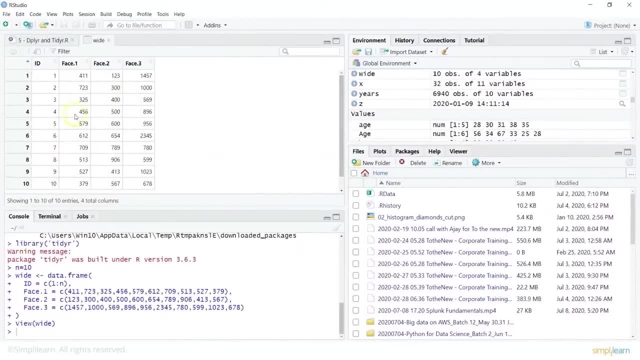 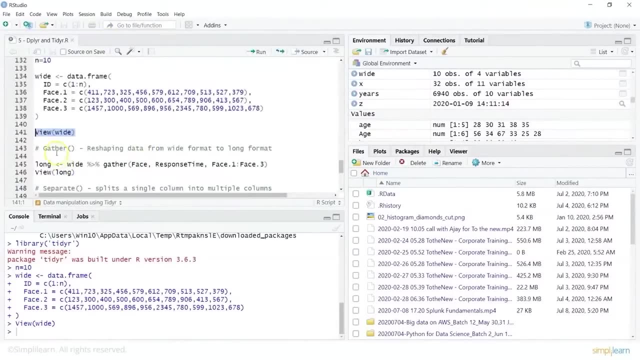 by just doing a view wide and that shows me the id column and it has phase dot 1, phase dot 2 and phase dot 3. now we can use our function. so, for example, we can work with gather, that is, reshaping the data from wide format. 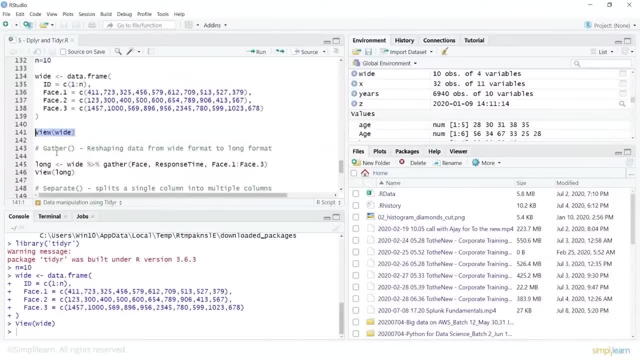 to long format and basically you can say stacking up multiple columns. so let's see how we do that here. I will call it long, I am working on wide, I am using the piping functionality and then I am using gather. so this one, I will say what will be the data which I 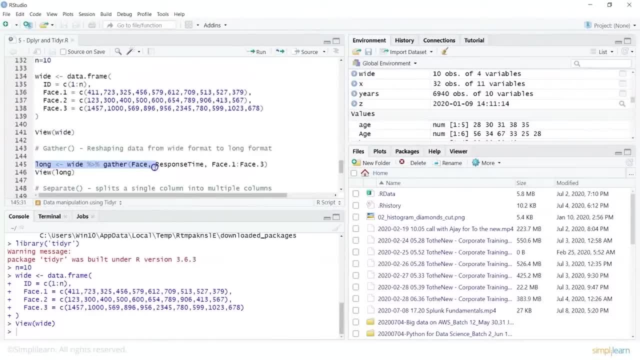 will use. so we are using wide as a data frame. then I am saying response time, so that will be basically one more column, and then you have your columns which you would want to basically stack. so I am saying from phase 1 to phase 3. so let's do this. 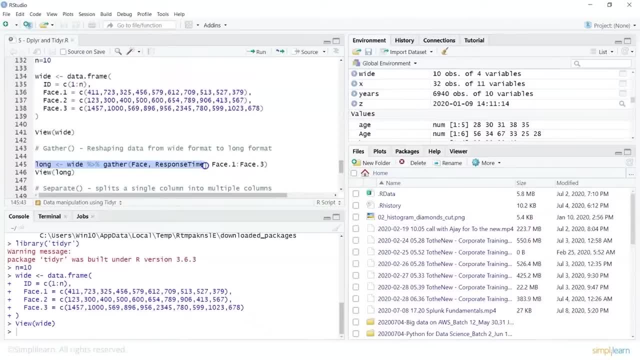 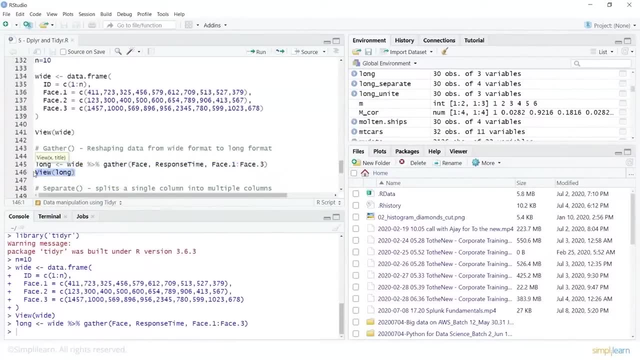 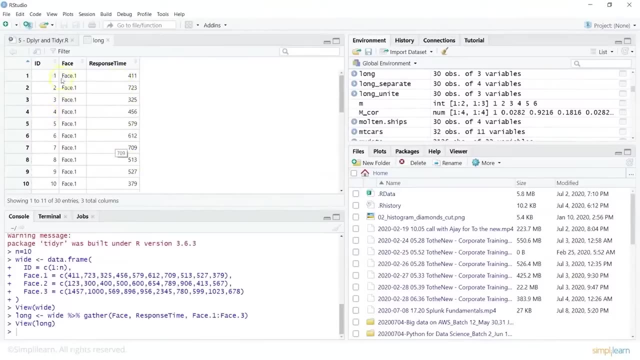 want to basically stack. so i am saying from face 1 to face 3. so let's do this. and once this is done, let's have a look at our variable long. so this one shows me that i have an id column, i have the response time column and i 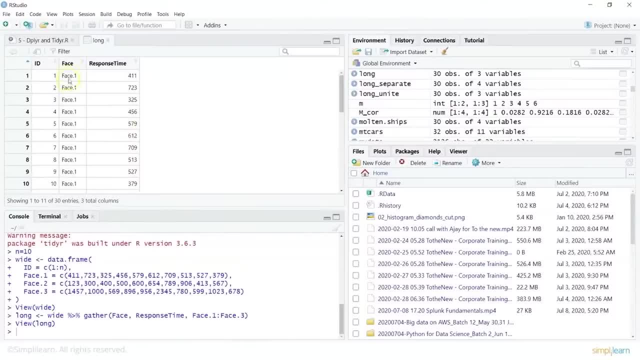 have the face column which we mentioned, and that basically has all the values stacked in. so you have face dot 1, face dot 2 and face dot 3. so all the columns are being stacked here. so all my data. so now i have totally 30 entries in this one. 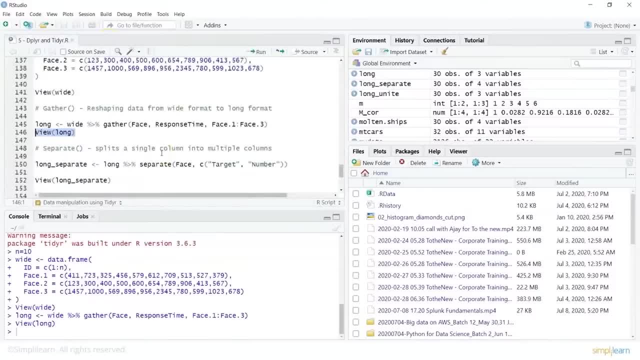 so this is basically using your gather function. now, sometimes we may want to use a separate function. now, separate function is basically splitting a single column into multiple columns, so which we would want to use when multiple variables are captured in a single variable column. okay, so let's look at an example. 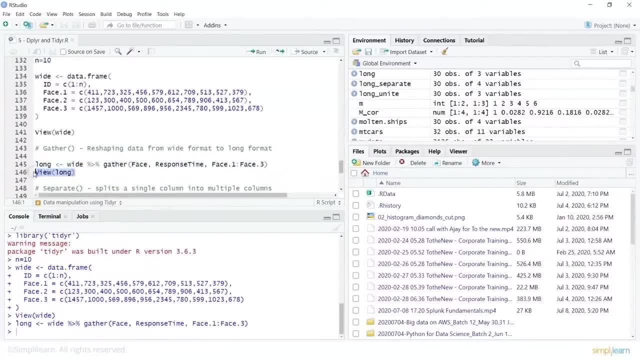 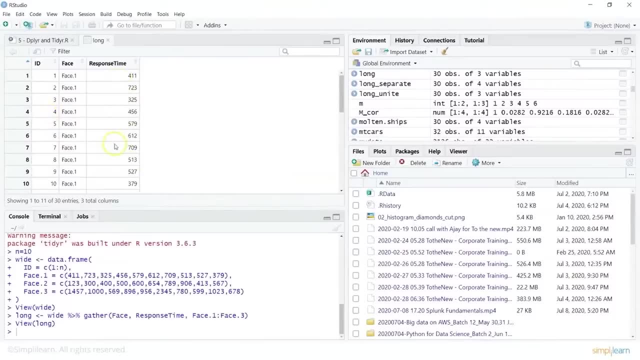 and once this is done, let's have a look at our variable long. so this one shows me that I have an id column, I have the response time column and I have the phase column, which we mentioned, and that basically has all the values stacked in. so you have phase. 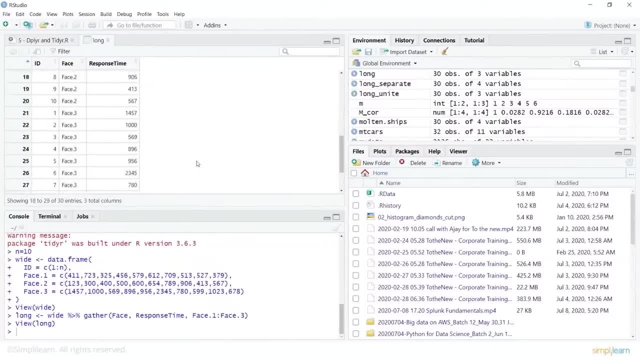 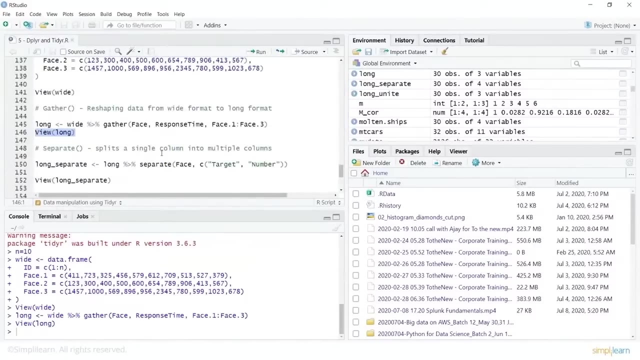 1, phase 2 and phase 3. so I have all the columns are being stacked here, so all my data. so now I have totally 30 entries in this one. so this is basically using your gather function. now sometimes we may want to use a separate function now. 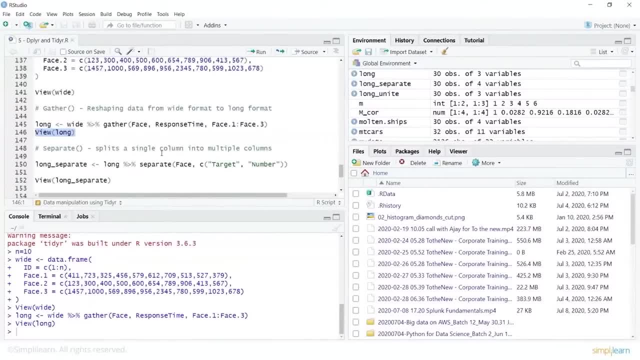 separate function is basically splitting a single column into multiple columns. so this is the function which we would want to use when multiple variables are captured in a single variable column. okay, so let's look at an example of this one. so let's say: long, separate, that's what. 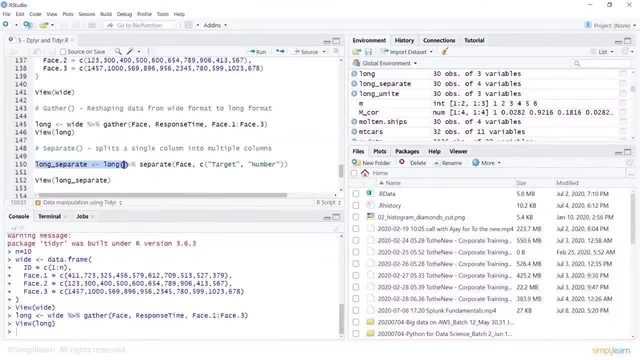 we will call, we will work on this long which has all the data stacked in as the columns we selected. then I am saying separate, I want the phase column. and then I would say, when I separate the columns, what are my column names? now I could also give: 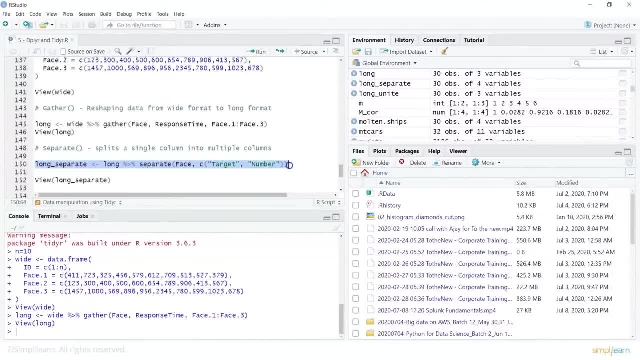 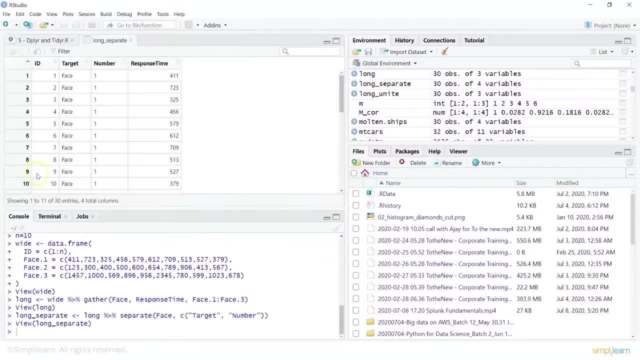 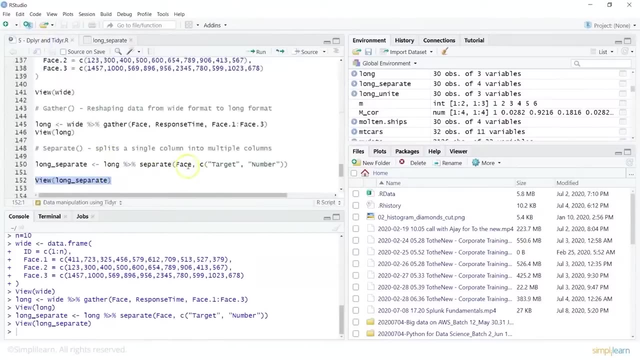 a separator by giving a comma, then mentioning the separator if that is required. so let's do this now. once this is done, let's have a look at our long separate. so what we see here is the column which we used. so we were doing a phase column. 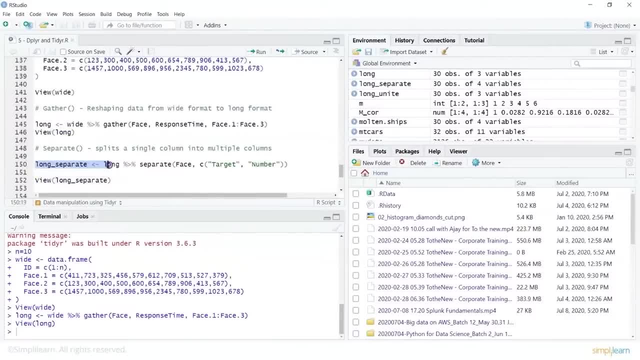 of this one. so let's say long, separate, that's what we will call. we will work on this long which has all the data stacked in as the columns we selected. then i am saying separate, i want the face column. and then i would say, when i separate the columns, what are my? 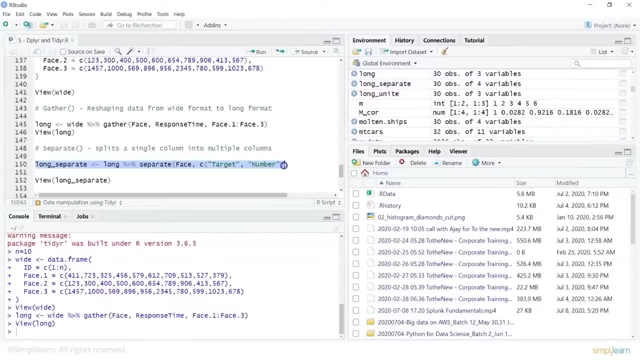 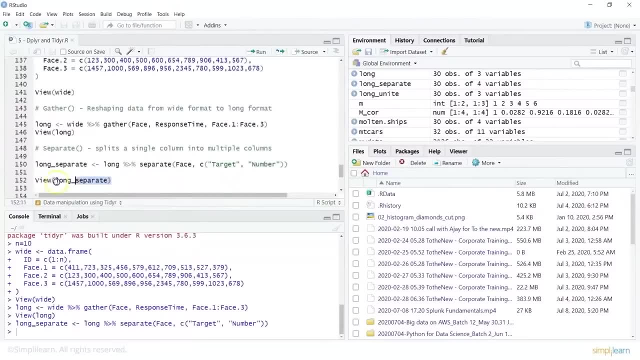 column names. now i could also give a separator by giving a comma and then mentioning the separator, if that is required. so let's do this now. once this is done, let's have a look at our long separate. so what we see here is the column which we used. 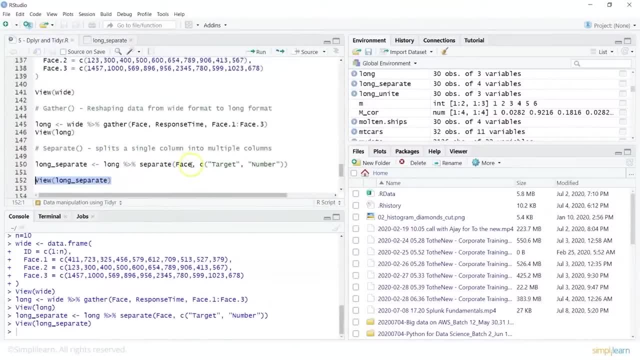 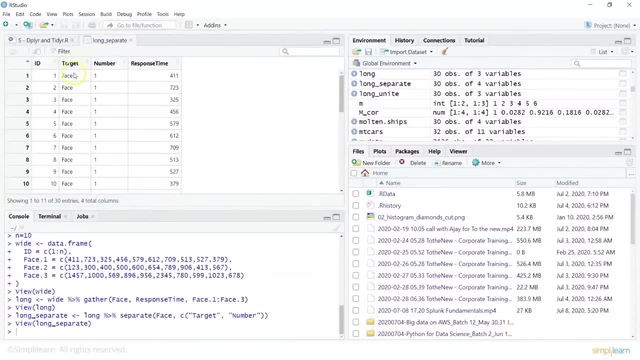 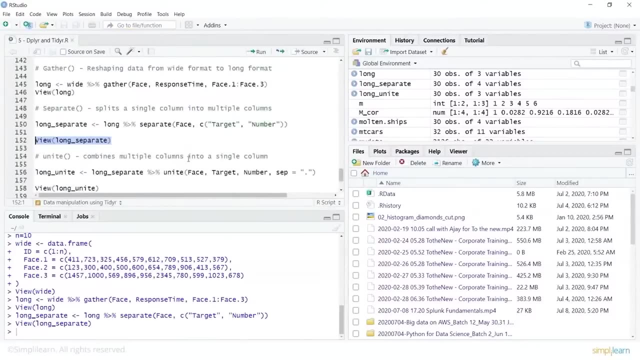 so we were doing a face column and that was to be split and we wanted to split it into target and number. so that's what we see here, so you have face being split into target and number and then you have the response time. so this is how you use the separate. 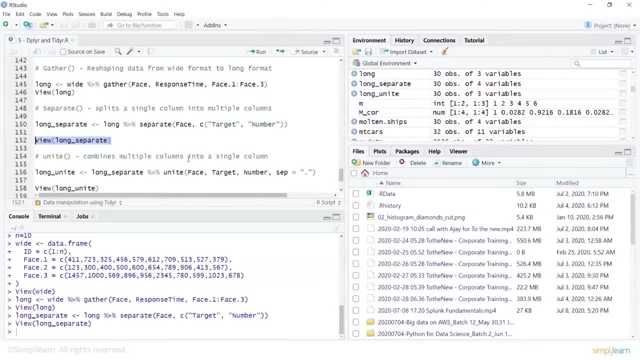 function. now there is also something called as unite function, which is basically a complementing of separate function. so it takes multiple columns and combines the elements to a single column. so for example, here we will call it long unite and we will take long separate, which was separating the data. 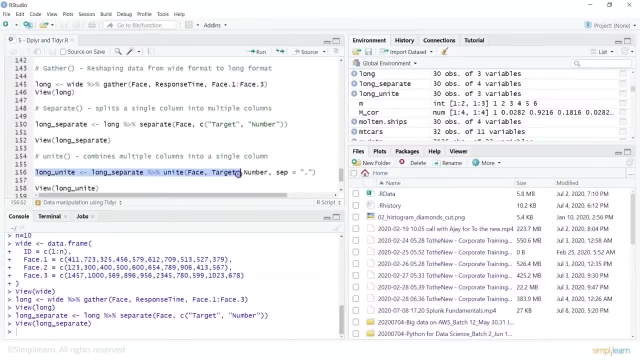 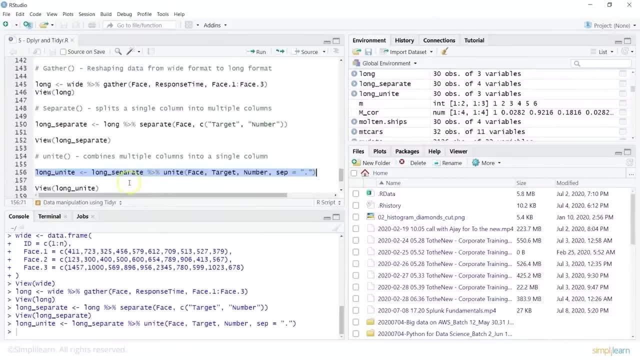 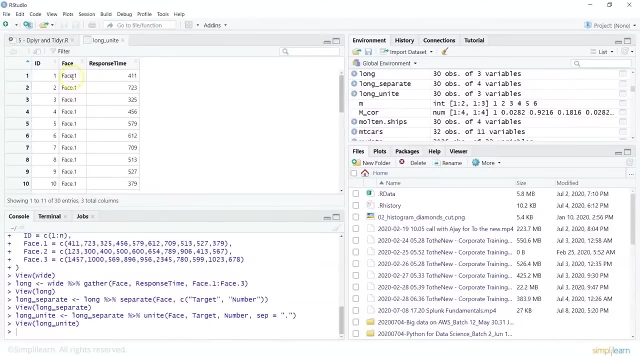 we want to unite, so we will take face target number and we want to have a separator between them. so let's basically do this. and now let's look at the result of this unite. so you see, you have the face and target merged together, so you have face dot. 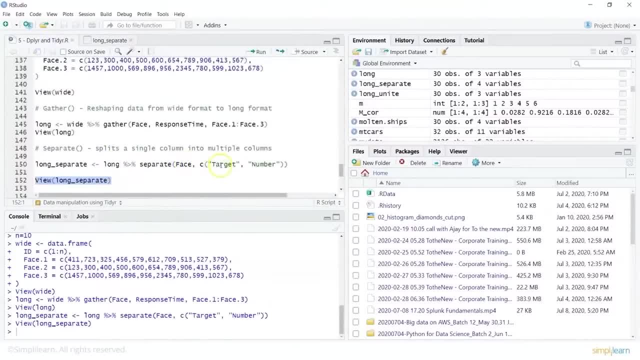 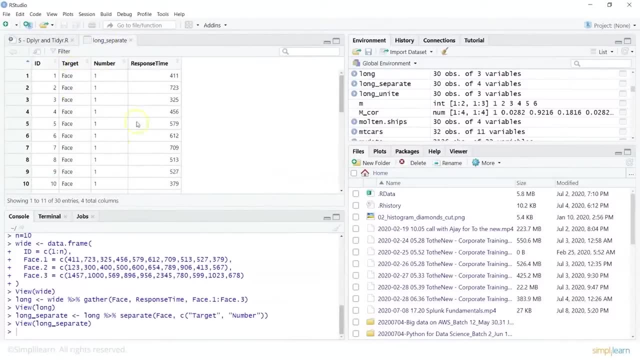 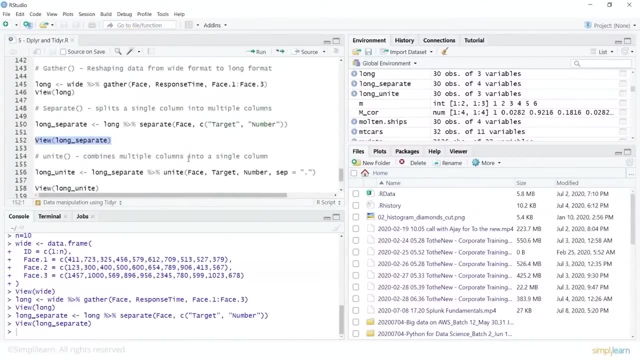 and that was to be split. and we wanted to split it into target and number. so that's what we see here. so you have phase being split into target and number and then you have the response time. so this is how you use the separate function. now there is also something called 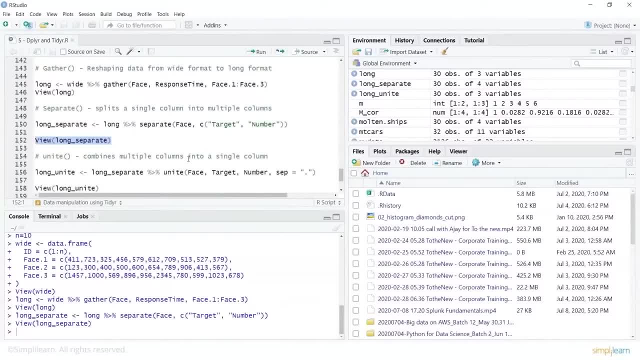 as unite function, which is basically a complementing of separate function. so it takes multiple columns and combines the elements to a single column. so, for example, here we will call it long unite and we will take long separate, which was separating the data we want to unite. so we will take 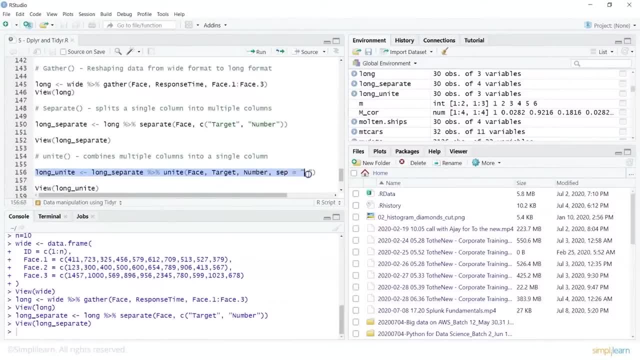 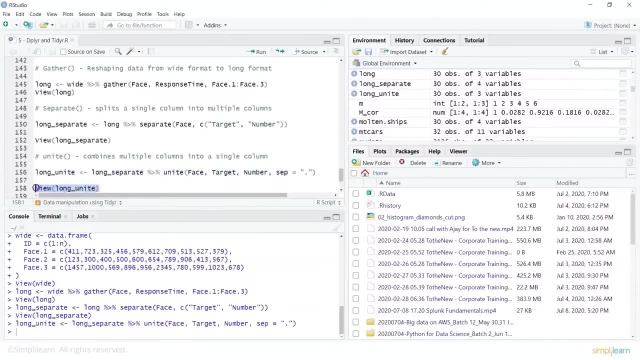 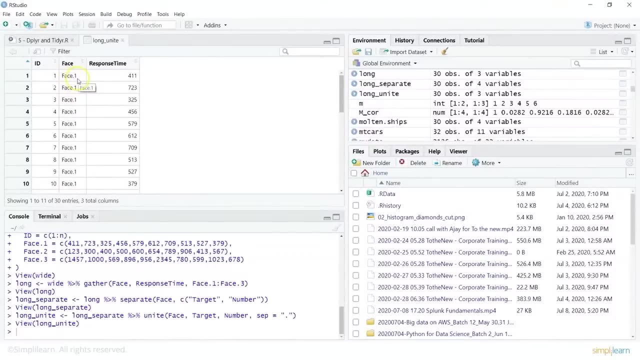 phase target number and we want to have a separator between them. so let's basically do this and now let's look at the result of this: unite, so you see, you have the phase and target merge together, so you have phase dot one. the separator is dot, as we have mentioned, and we have united. 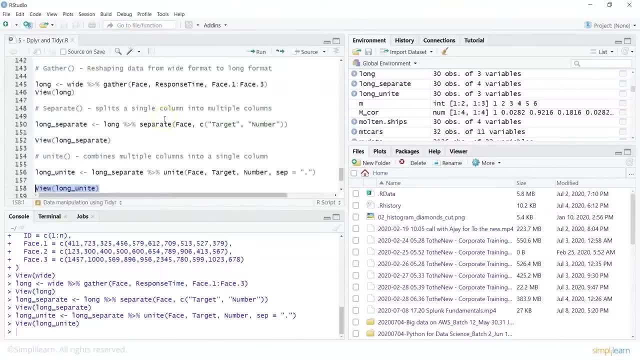 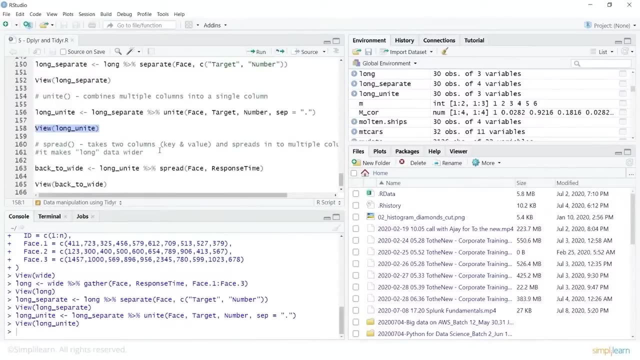 multiple columns. so this is one more function of your tidyR which helps you basically tidy up your data or put it in a particular way now. then you have your spread function and this is basically for unstacking. so that is if you have, if you would want to convert a stack. 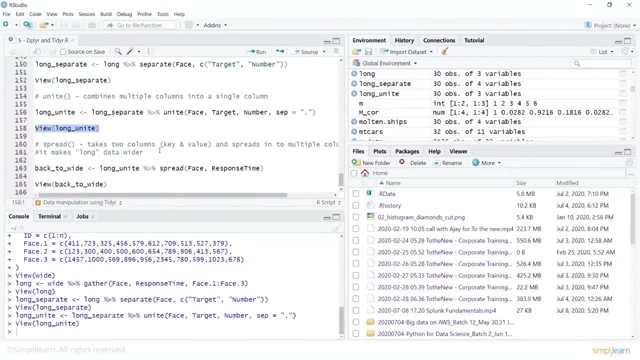 to data or if you would want to unstack the data which is of same attributes, spread can be used so that you can spread the data across multiple columns. so it will take two columns, say key and value, and spread it into multiple columns. so it makes long data wider. 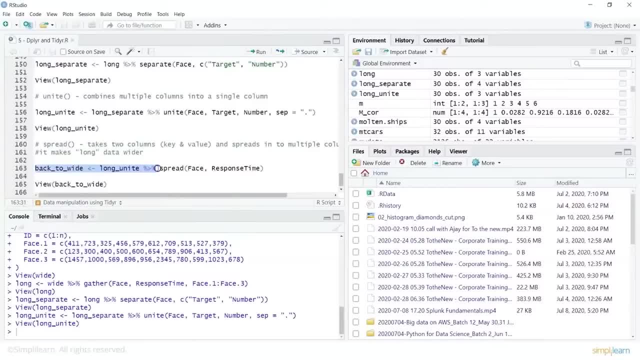 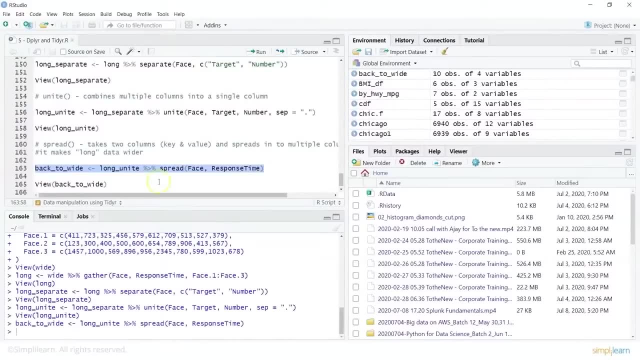 so we can look at this one. we will say long unite. I am using the typing, I will use the spread function, I will work on the phase column and response time and let's do this and then let's do a view on this so it tells me our 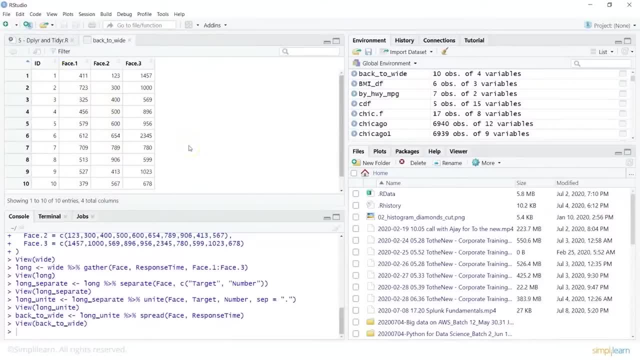 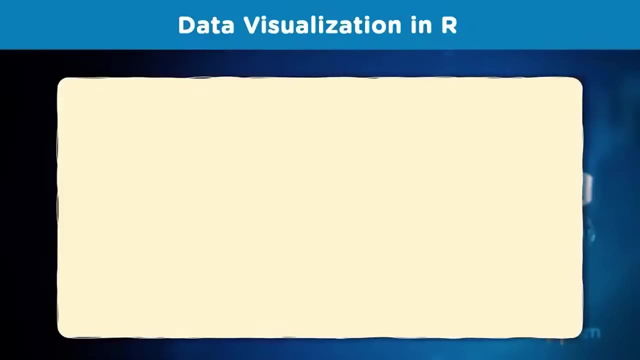 data is back in the shape as it was in the beginning. so these are four functions which are very helpful when we work with tidyR package. so let's learn about visualization, and here we will learn about R, which can be used for your visualization. now one thing. 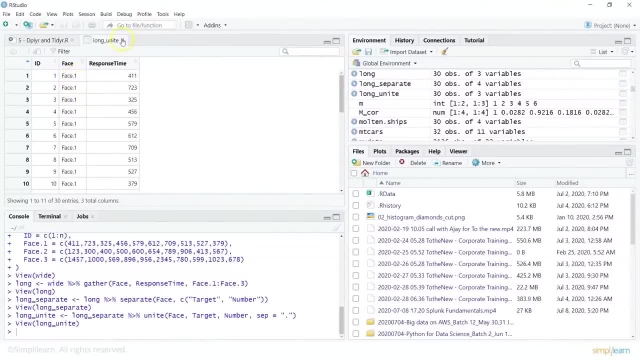 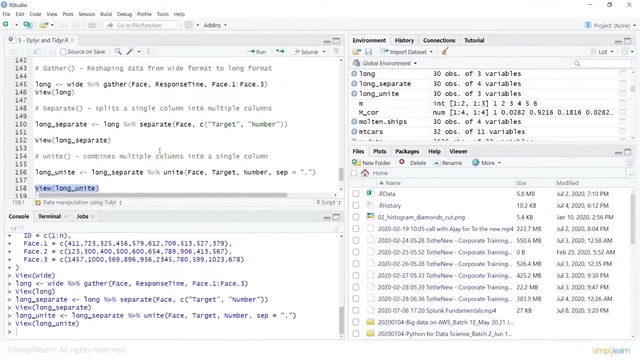 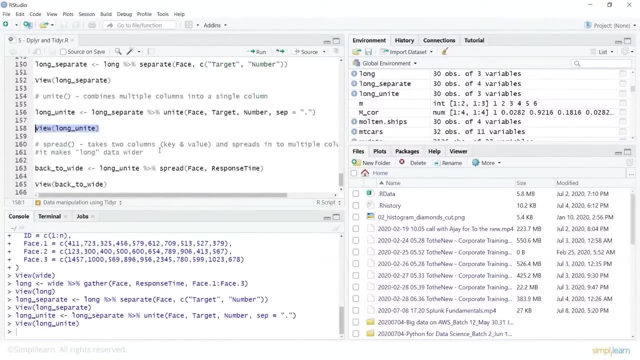 one. the separator is dot, as we have mentioned, and we have united multiple columns. so this is a more function of your tidyR, which helps you basically tidy up your data, or put it in a particular way. now then you have your spread function, and this is basically for unstacking. 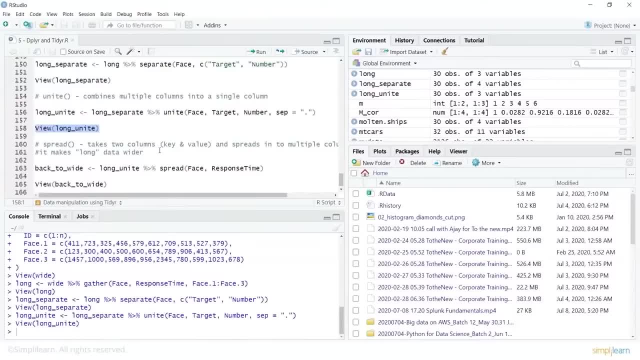 so that is, if you have, if you would want to convert a stack to data or if you would want to unstack the data which is of same attributes, spread can be used so that you can spread the data across multiple columns. so it will take two columns. 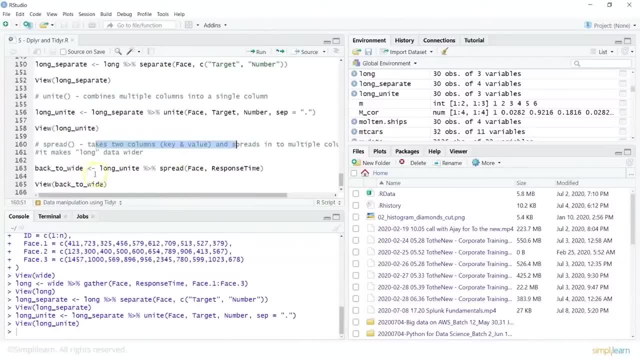 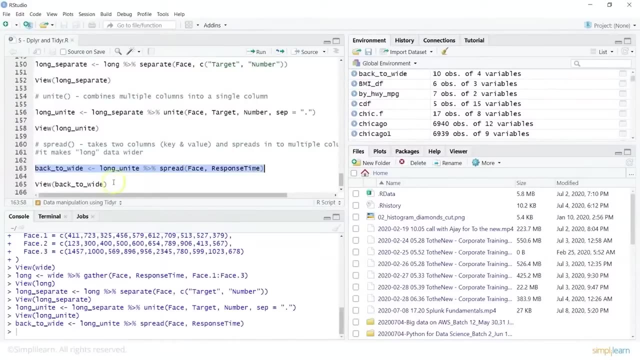 say key and value and spread it into multiple columns so it makes long data wider. so we can look at this one. we will say long unite. I am using the piping, I will use the spread function, I will work on the face column and response time and let's do this and 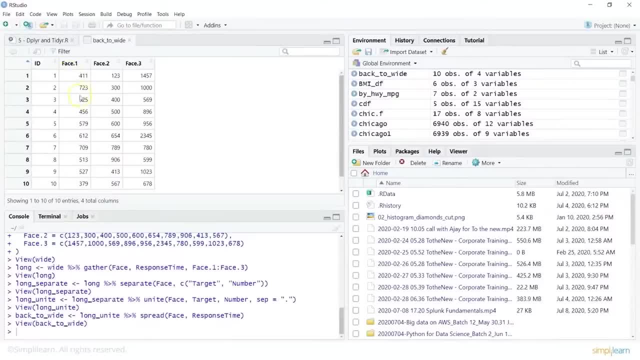 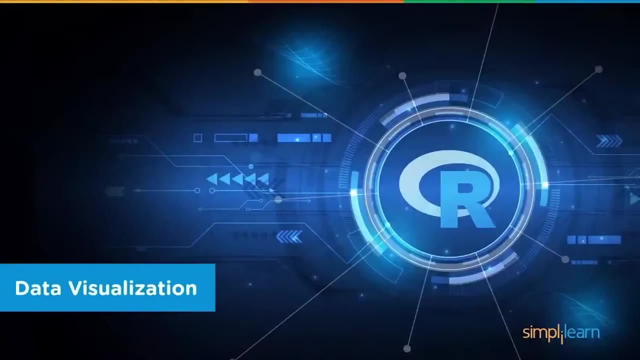 then let's do a view on this. so it tells me our data is back in the shape as it was in the beginning. so these are four functions which are very helpful when we work with tidy R package. so let's learn about visualization, and here we will learn. 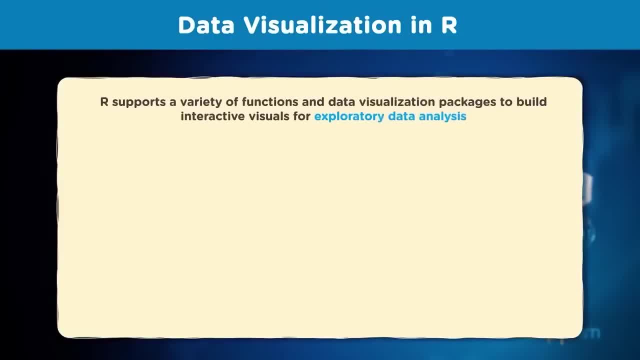 about R, which can be used for your visualization. now, one thing which we need to understand is because of our ability to see patterns, which is highly developed, we can understand the data better if we can visualize it. so the efficient way or effective way to understand what is in our data, 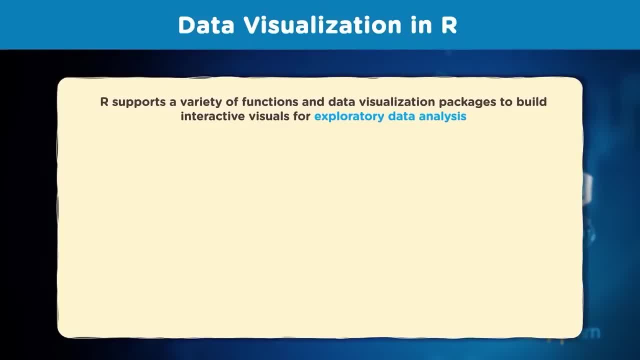 or what we have understood in our data. we should or we can use graphical displays. that is your data visualization. so there are actually two types of data visualizations. so you have exploratory data visualization, which helps us to understand the data, and then you have explanatory visualization. 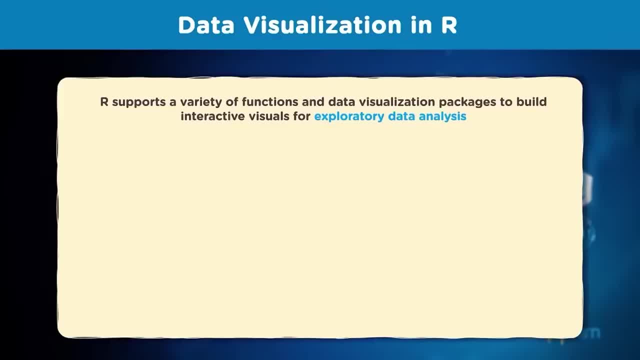 which helps us to share our understanding with others. so when you talk about R, R provides various tools and packages to create data visualizations and which can be used for both kind of data analysis or both kind of visualizations. so, when you talk about exploratory data visualization, 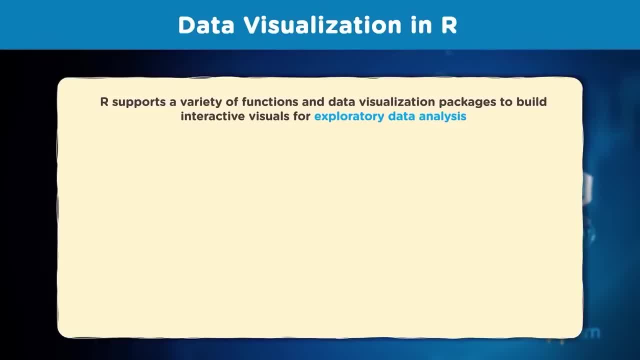 the key is to keep all the potentially relevant details together. now, the objective when we talk about exploratory data analysis is to help you see what is in your data, and the main question is: how much details can we interpret? now, when you talk about different functions, which we 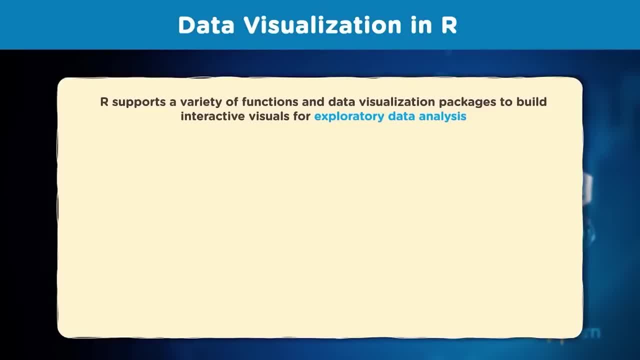 which we need to understand is because of our ability to see patterns, which is highly developed. we can understand the data better if we can visualize it. so the efficient way or effective way to understand what is in our data, or what we have understood in our data, we should or 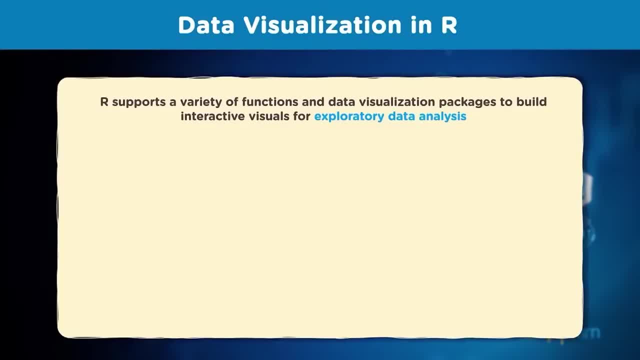 we can use graphical displays. that is your data visualization. so there are actually two types of data visualizations. so you have exploratory data visualization, which helps us to understand the data, and then you have explanatory visualization, which helps us to share our understanding with others. so when you talk about R, 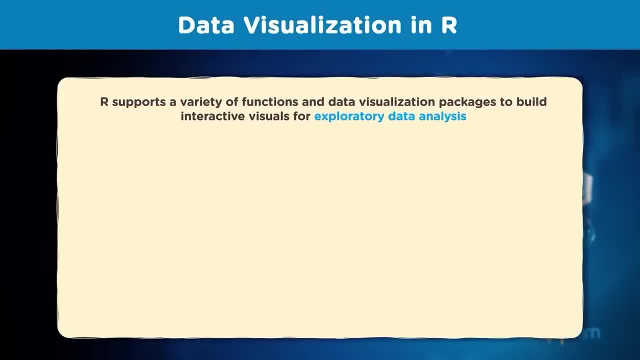 R provides various tools and packages to create data visualizations and which can be used for both kind of data analysis or both kind of visualizations. so when you talk about exploratory data visualization, the key is to keep all the potentially relevant details together. now the objective. when we talk about 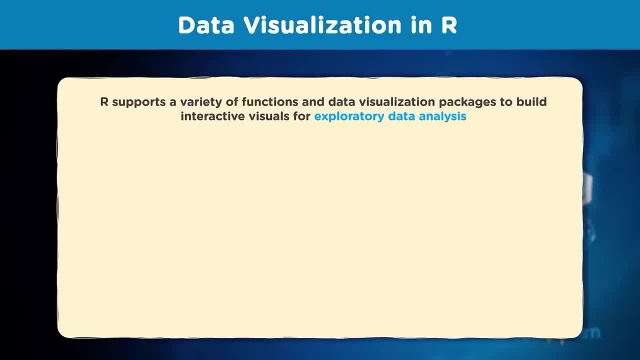 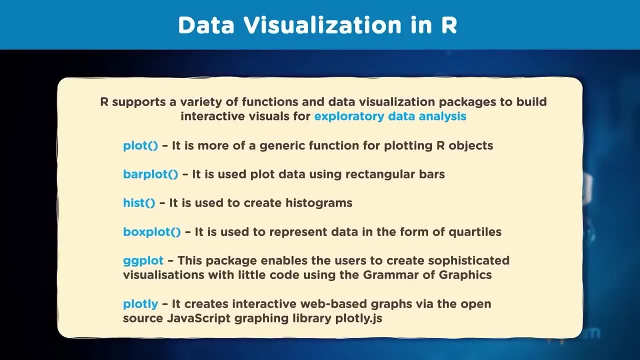 exploratory data analysis is to help you see what is in your data, and the main question is: how much details can we interpret? now, when you talk about different functions which we see here, such as plot, which is more for a generic plotting, you have bar plot, which is 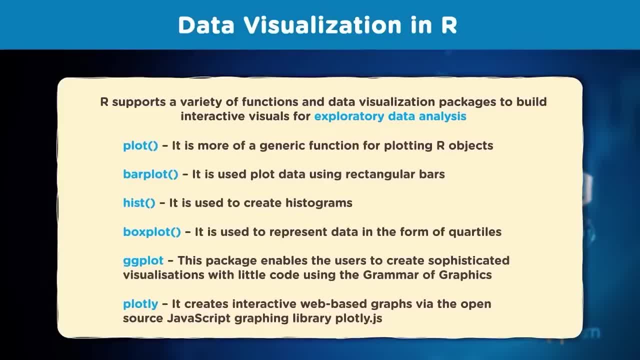 used to plot data using rectangular bars or you can say, creating bar charts. you have histogram or hist function to create histograms, where you look at the frequency of the data or basically used to look at the central tendency of the data. you have box plot, which is used to represent data in the 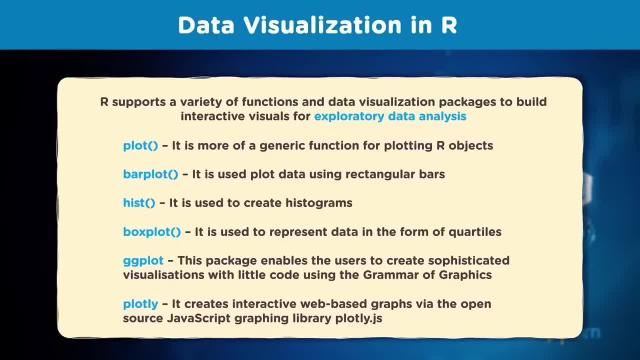 form of quartiles. you have ggplot, which is a package which enables the user to create sophisticated visualizations with the little code using the grammar of graphics. and then you have plotly. or plotly, it creates interactive web based graphs via the open source javascript graphing library. 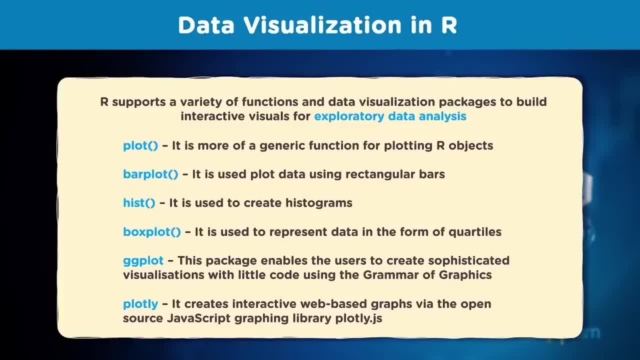 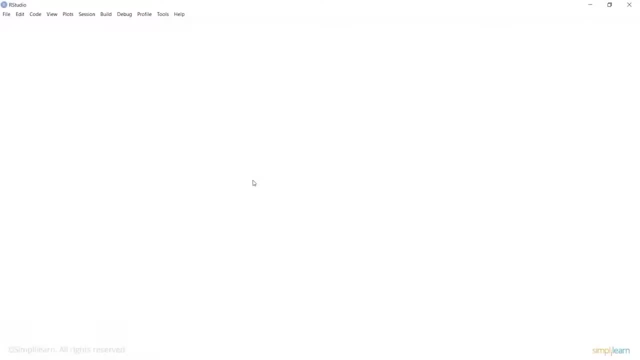 now, before we see some examples here, lets also talk about when you talk about plotting. lets also try to understand what kind of plots you can have and what kind of techniques you have. so let me open up my R studio here now. for example, i can pull out a particular data. 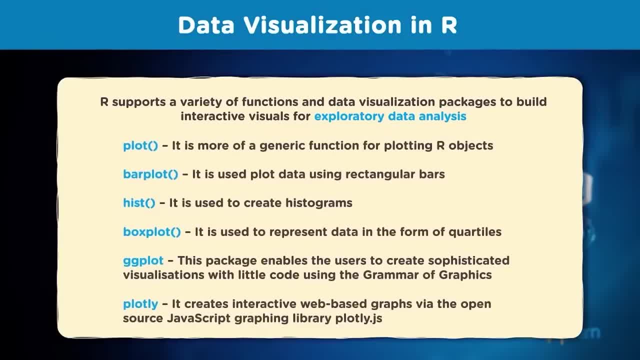 see here, such as plot, which is more for a generic plotting. you have bar plot, which is used to plot data using rectangular bars, or you can say creating bar charts. you have histogram or hist function to create histograms where you look at the frequency of the data, or basically. 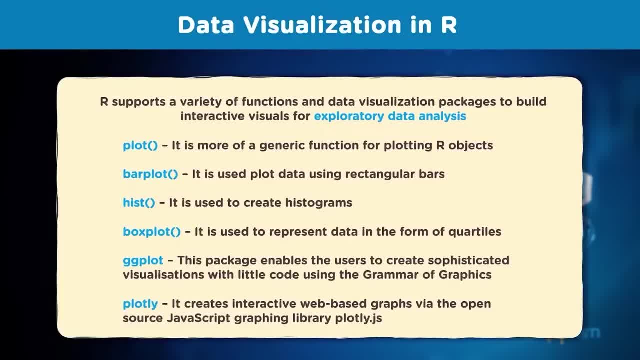 used to look at the central tendency of the data. you have box plot, which is used to represent data in the form of quartiles. you have gg plot, which is a package which enables the user to create sophisticated visualizations with the little code, using the grammar of graphics. 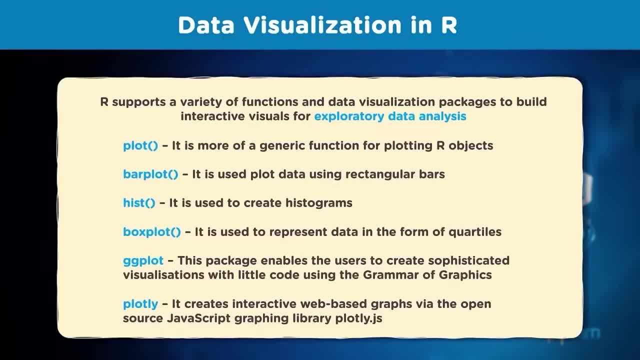 and then you have plotly, or plotly, it creates interactive web based graphs via the open source javascript graphing library. now, before we see some examples here, lets also talk about when you talk about plotting. lets also try to understand what kind of plots you can have. 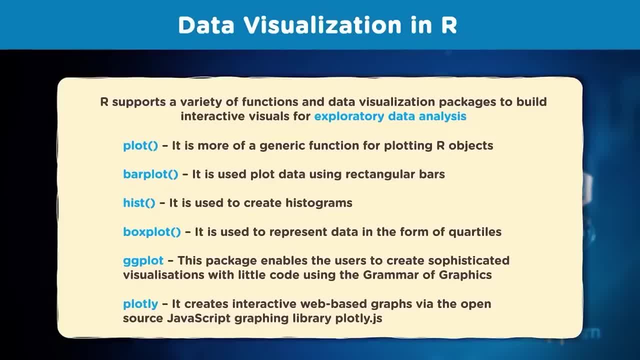 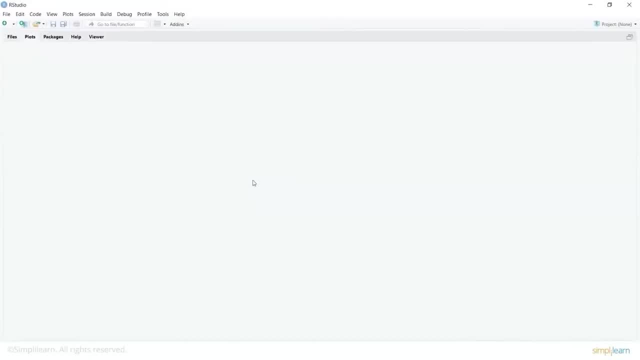 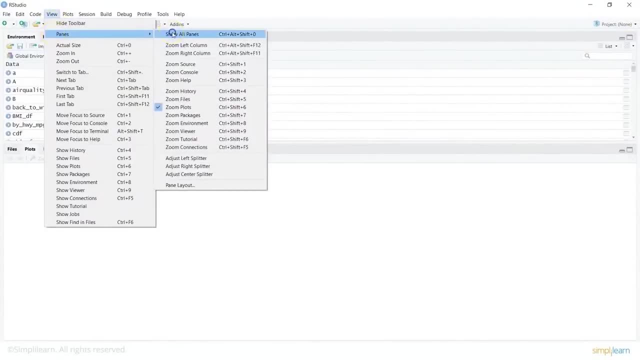 and what kind of techniques you have. so let me open up my R studio here now. for example, i can pull out a particular data set and lets look at this one. so here i can look at all the panes and that shows me the information. now what i can do is 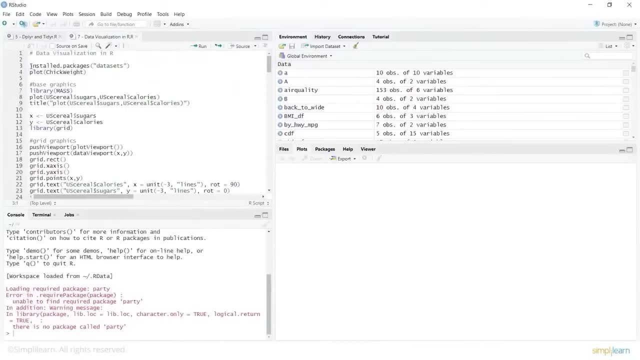 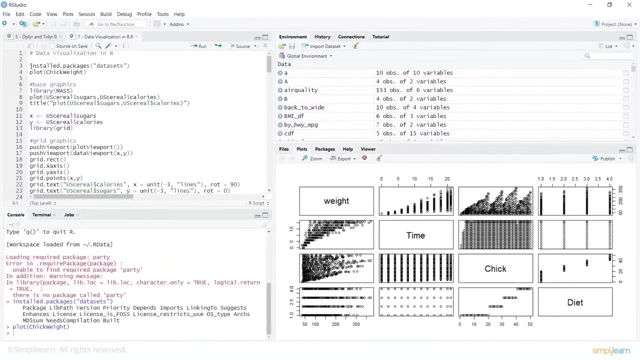 i can install and get the inbuilt data sets and then i can simply do a plot wherein i am doing a plot on chick weight data set. so lets see what does that show? it summarizes the relationship between four variables in chick weight data frame, which is in R's built in data. 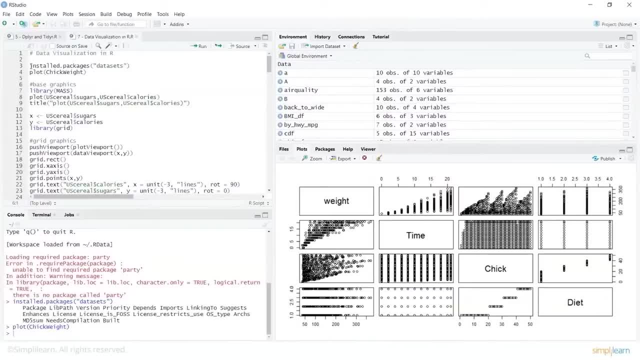 set package. now, from these plots we can see, for example, weight varies systematically over time. you can also see that chicks were assigned to four different diets. now when we talk about explanatory data analysis or visualization that shows others what we found in the data, this means we need to make. 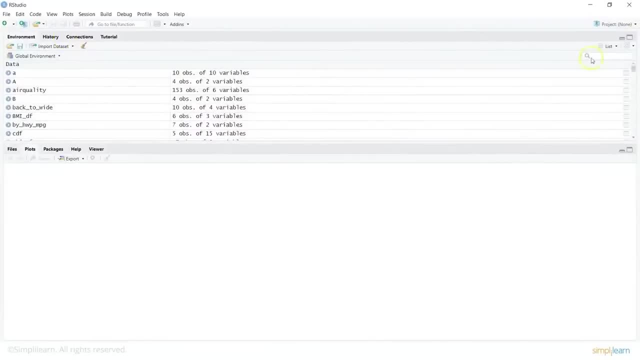 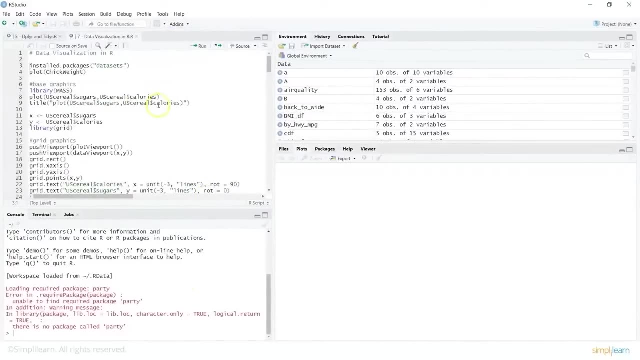 set, and lets look at this one. so here i can look at all the panes and that shows me the information. now what i can do is i can install and get the inbuilt data sets and then i can simply do a plot. where in i am doing a plot on? 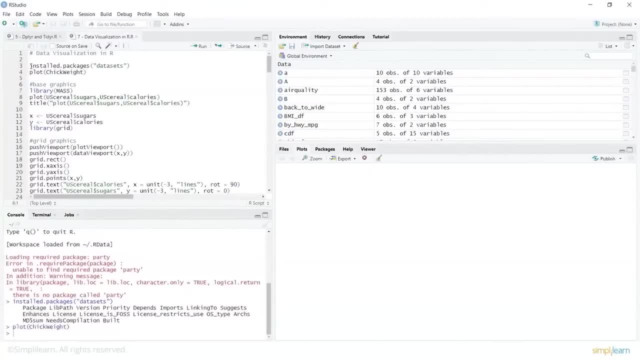 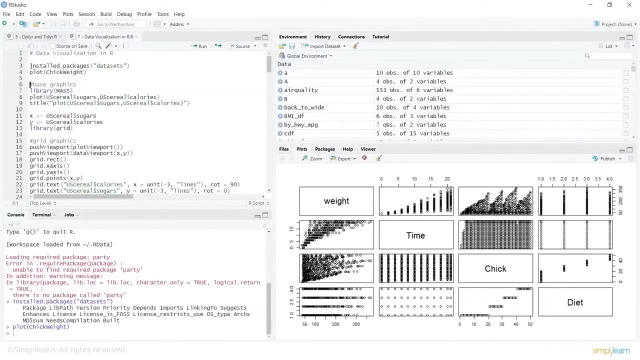 chick weight data set. so lets see what does that show? it summarizes the relationship between four variables in chick weight data frame, which is in R's built in data set package. now from these plots we can see, for example weight varies systematically over time. you can also see: 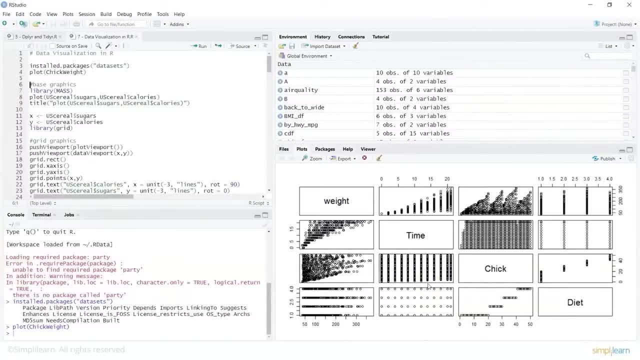 that chicks were assigned to four different diets. now we talk about explanatory data analysis or visualization that shows others what we found in the data. this means we need to make some editorial decisions: what features we would want to highlight for emphasis, what features are distracting or confusing and you want them to be eliminated? 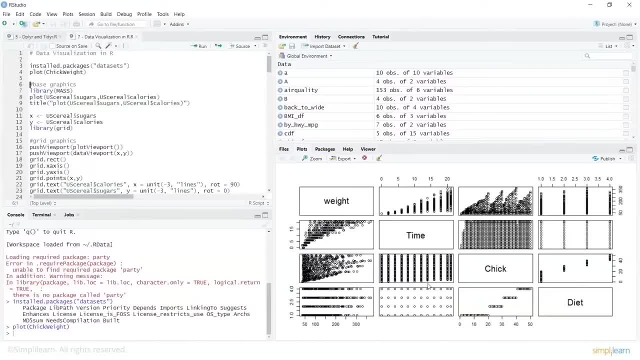 right. so there are different ways of doing it. now, when you talk about your graphics or visualizations, you have, i would say, three different types, or you can say four, so you have the base graphics, which is easiest to learn. now, here we are having an example of base graphics, where 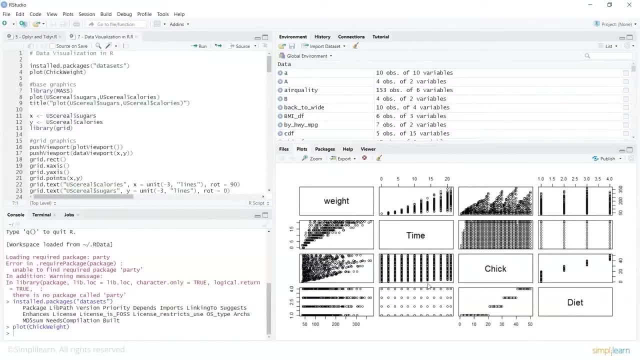 i can use the base graphics, i can get a data set using library. then i can simply create using plot function to generate a simple scatter plot of calories with sugar from US serial data frame in the mass package and then i can give it a title. so this is basically a simple 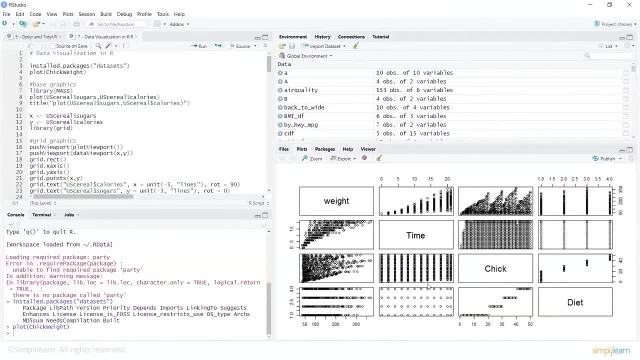 some editorial decisions, what features we would want to highlight for emphasis, what features are distracting or confusing and you want them to be eliminated, right? so there are different ways of doing it. now, when you talk about your graphics or visualizations, you have, i would say, three different types. 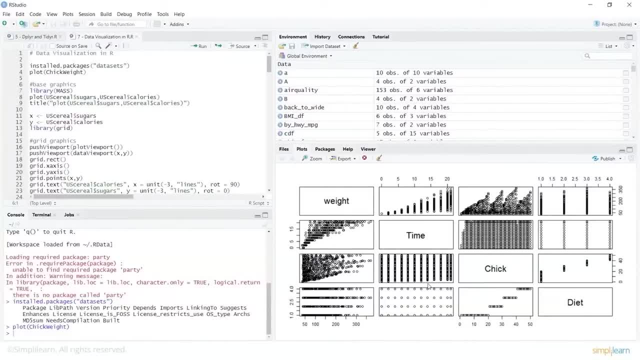 or you can say four, so you have the base graphics, which is easiest to learn. now, here we are having an example of base graphics where i can use the base graphics. i can get a data set using library. then i can simply create using plot function to a generate a simple 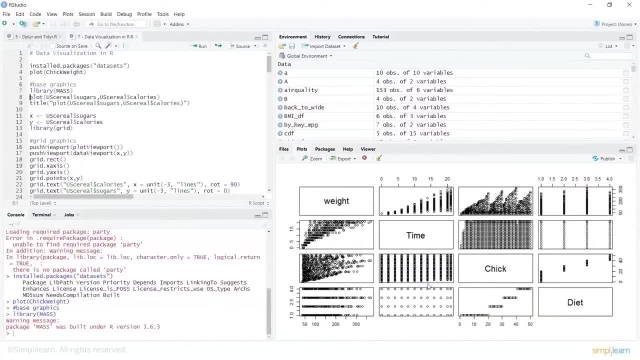 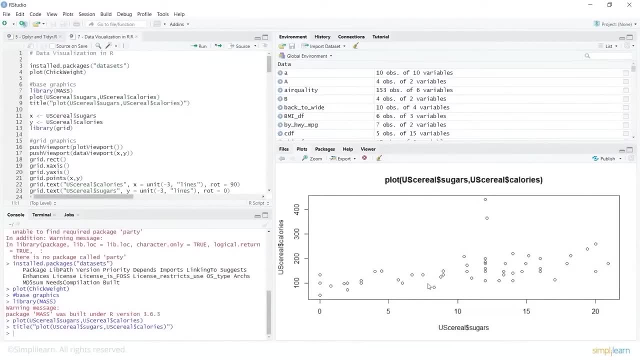 scatter plot of calories with sugar from us serial data frame in the mass package and then i can give it a title. so this is basically a simple example of base graphics. now you also have what we call as grid graphics, which is powerful set of modules for building. 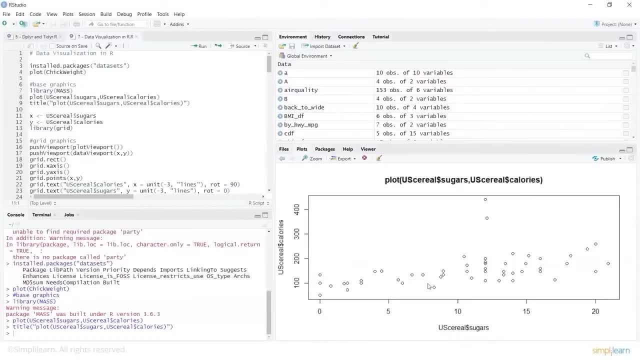 other tools. now you also have latest graphics, which is general purpose system based on grid graphics, and then you have your gg plot 2, which is implements grammar of graphics and is based on grid graphics. so you have different ways now here, since i already have used library and 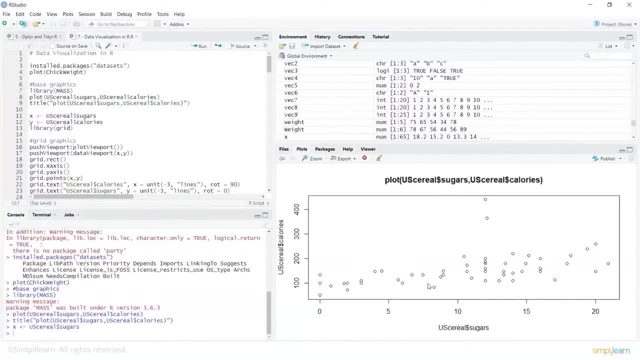 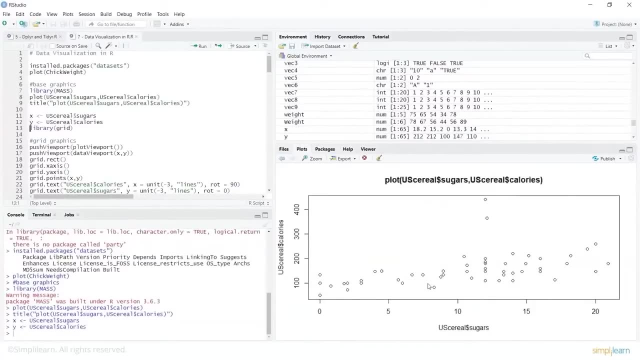 i have the data set. i can just do a x so i can assign the sugar related values to x and calories related value to y. then i can use one more, which is library function and calling in grid. now i can basically use functions such as push viewport if i would. 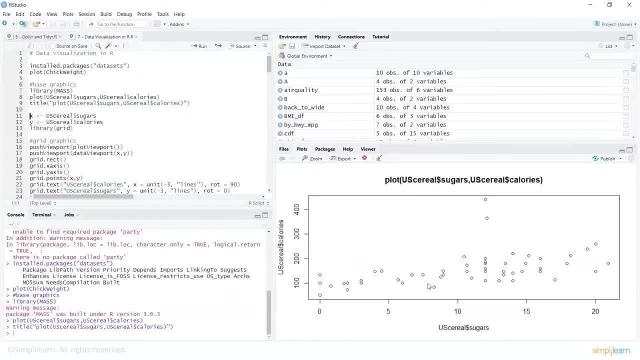 example of base graphics. now you also have what we call as grid graphics, which is powerful set of modules for building other tools. now you also have latest graphics, which is general purpose system based on grid graphics. and then you have your ggplot2, which implements grammar of graphics and is 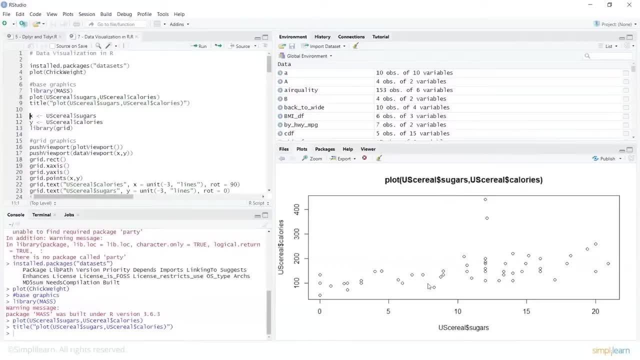 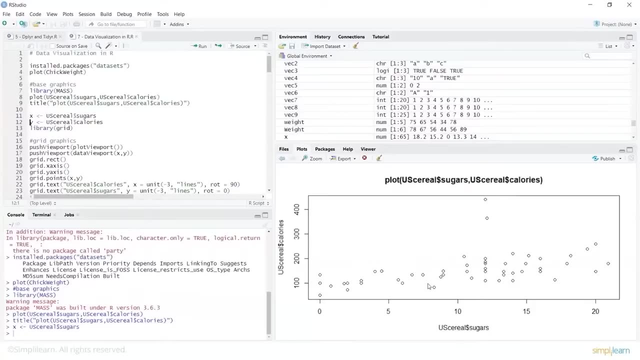 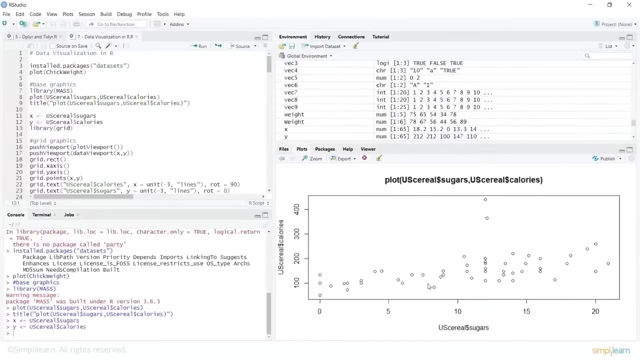 based on grid graphics. so you have different ways now here. since i already have used library and i have the data set, i can just do a x so i can assign the sugar related values to x and calories related value to y. then i can use one more, which. 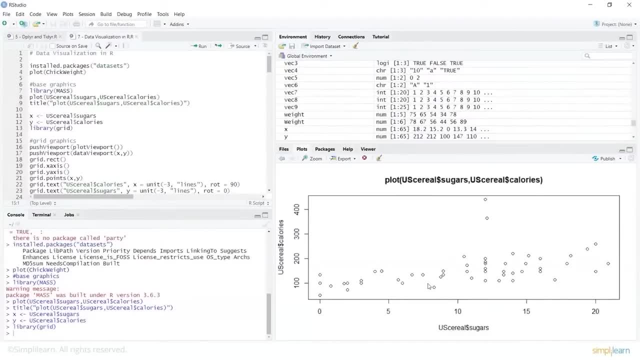 is library function and calling in grid. now i can basically use functions such as pushviewport if i would want to create a plot using your grid graphics, to create the similar kind of plot which we created using base graphics, but this will give you much more power than base graphics. 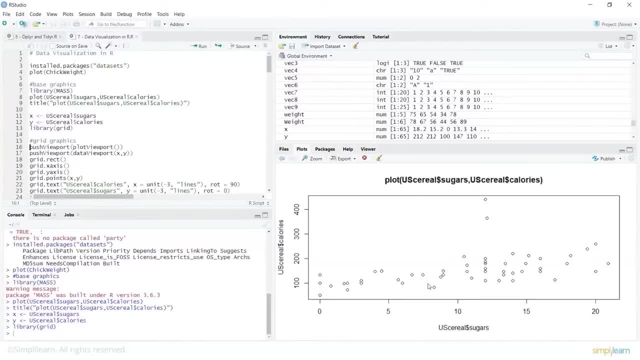 it will have a steep learning curve but it is usually useful. so i can do this. where i am saying pushviewport, then i can basically say i would want to have a data viewport. i would say different functions of your grid package. so i am saying rectangle, you have x axis, y axis. 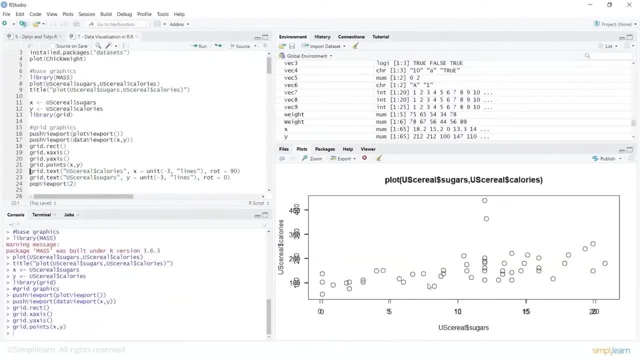 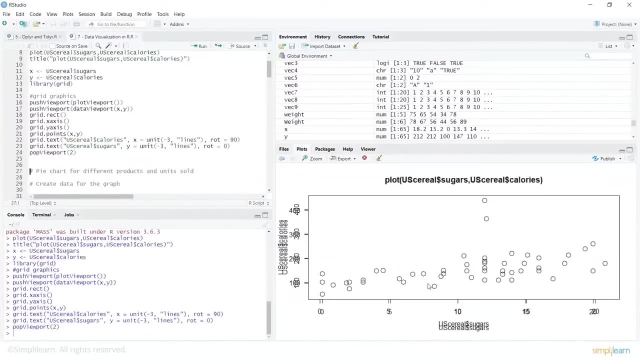 given some points here and then basically, you can add details to the graph by giving the names to the columns and you can basically create a simple grid graphics based plot here now there are different other options which we can use to create plots. now, before we go into understanding, 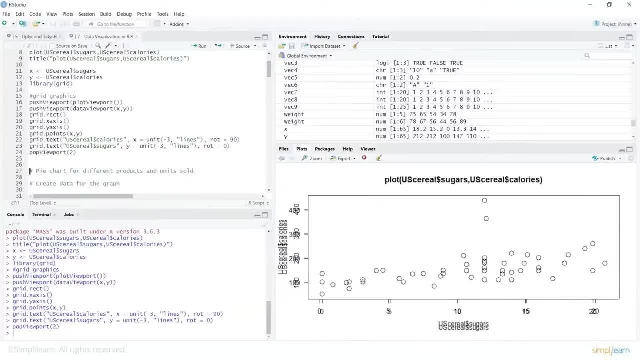 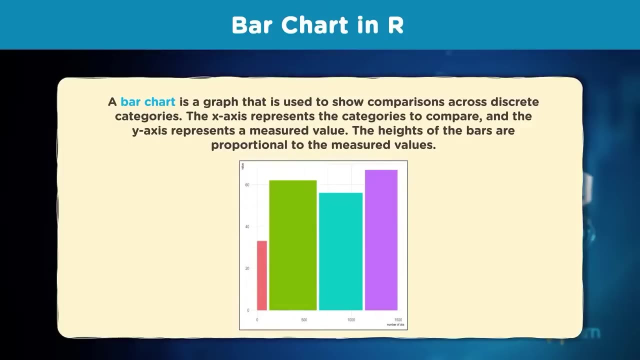 how you create plots. let me just give you a brief on what are the different kind of plots and how they can be used. so here we will look at these different plots. now, for example, we have a bar chart, which is a graph which shows comparisons across discrete categories. 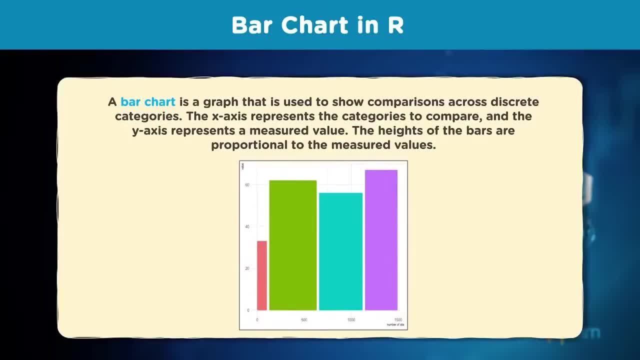 so you have x axis, which will show the categories being compared, and y axis, which represents a measured value, and height of the bars are proportional to measured values. now, to create different kind of charts, you can use ggplot, which is a package for creating graphs in R. 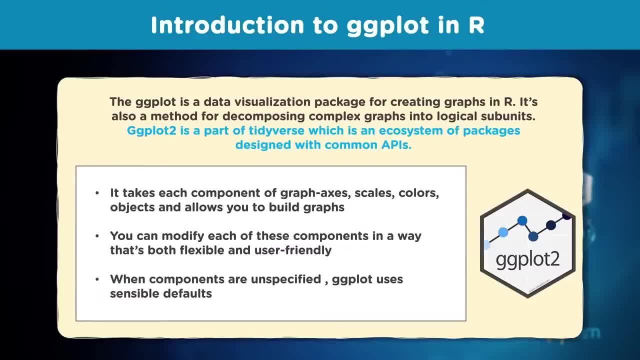 it is basically method of thinking about and decomposing complex graphs into logical subunits, and that is a part of tidyverse ecosystem, so it takes each component of graph accesses. you can give scales, you can give colors, you can give the objects and you can build graphs. 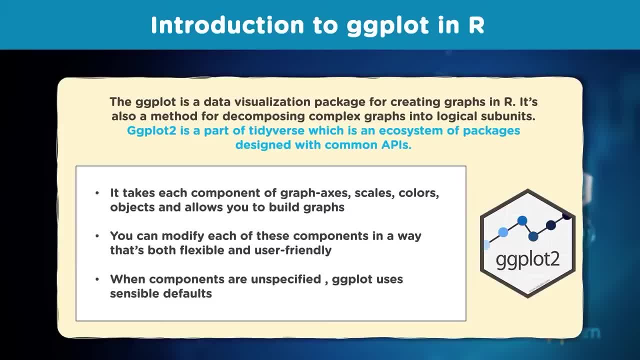 on particular data. you can modify each of those components in a way that is more flexible and user friendly. you can. if you are not providing details for the components, then ggplot will use sensible defaults, and this basically makes it a powerful and a flexible tool. now here are 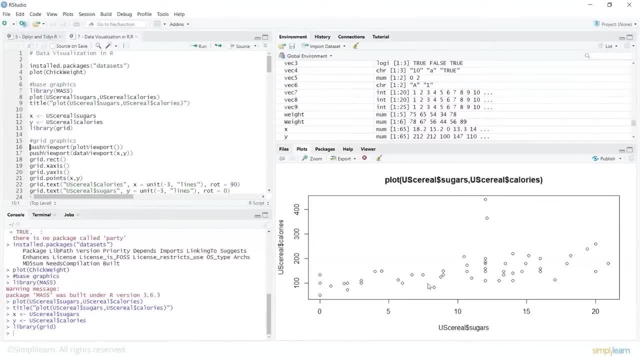 want to create a plot using your grid graphics to create the similar kind of plot which we created using base graphics, but this will give you much more power than base graphics. it will have a steep learning curve, but it is usually useful. so i can do this where i am saying 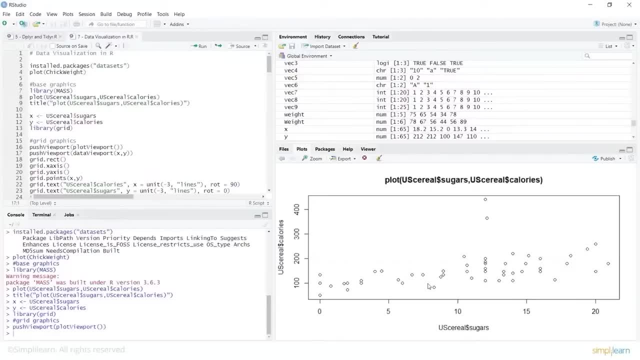 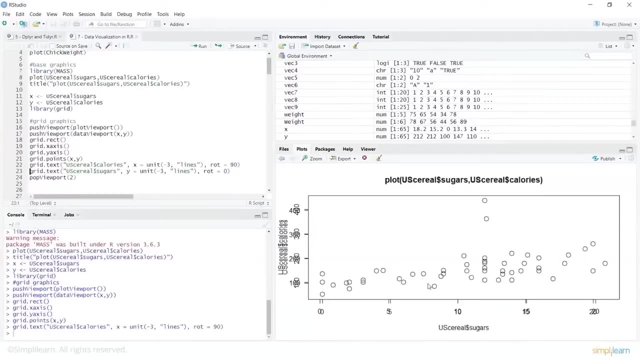 push viewport. then i can basically say i would want to have a data viewport. i would say different functions of your grid package. so i am saying rectangle, you have x axis, y axis, given some points here, and then basically you can add details to the graph by giving the names. 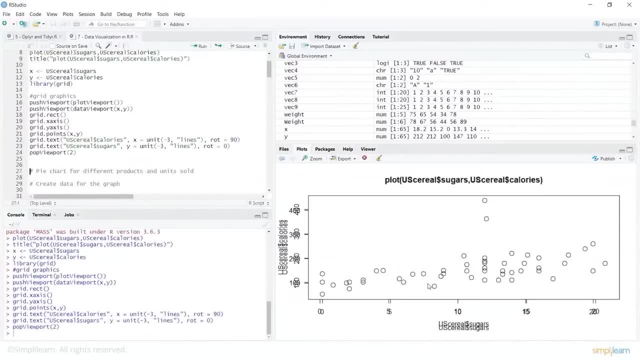 to the columns and you can basically create a simple grid graphics based plot here. now there are different other options which we can use to create plots. now, before we go into understanding how you create plots, let me just give you a brief on what are the different kind of plots and 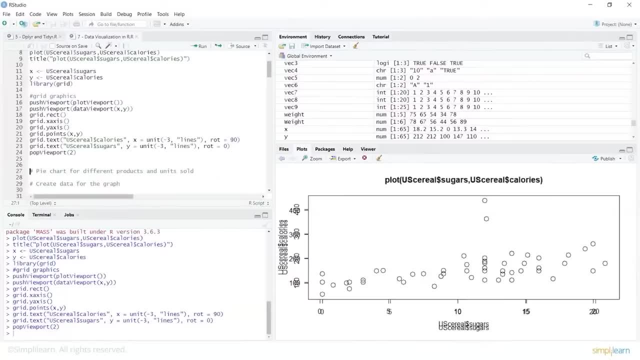 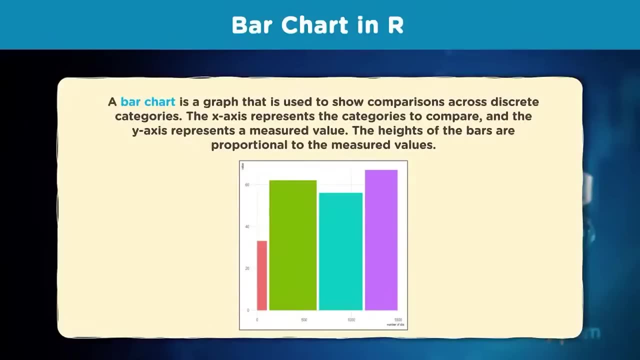 how they can be used. so here we will look at these different plots. now, for example, we have a bar chart, which is a graph which shows comparisons across discrete categories. so you have x axis which will show the categories being compared, and y axis which represents a measured value and height of 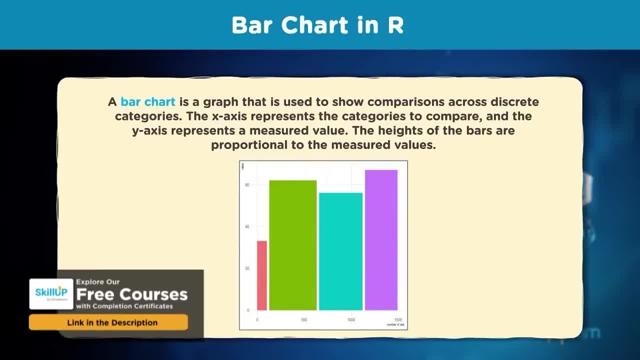 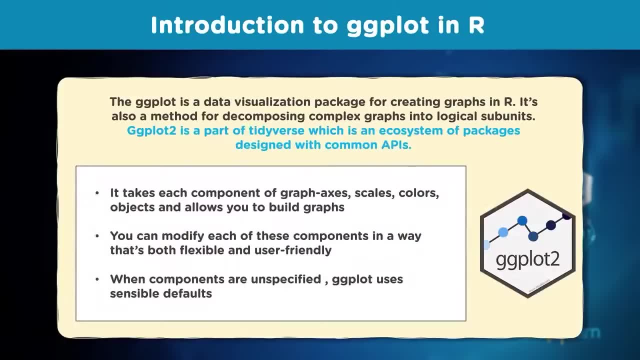 the bars are proportional to measured values. now, to create different kind of charts, you can use ggplot, which is a package for creating graphs in R. it is basically method of thinking about and decomposing complex graphs into logical subunits, and that is a part of tidyverse ecosystem. 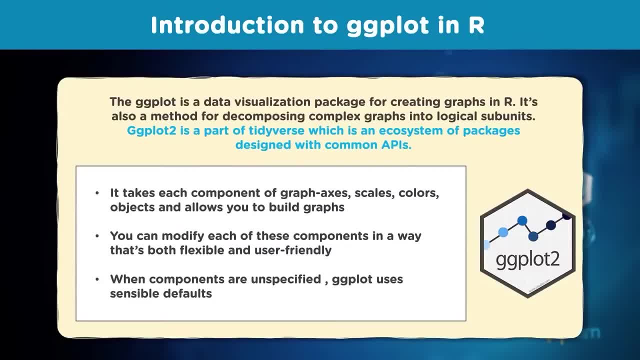 so it takes each component of graph accesses. you can give scales, you can give colors, you can give the objects and you can build graphs on particular data. you can modify each of those components in a way that's more flexible and user friendly. you can if you are not providing. 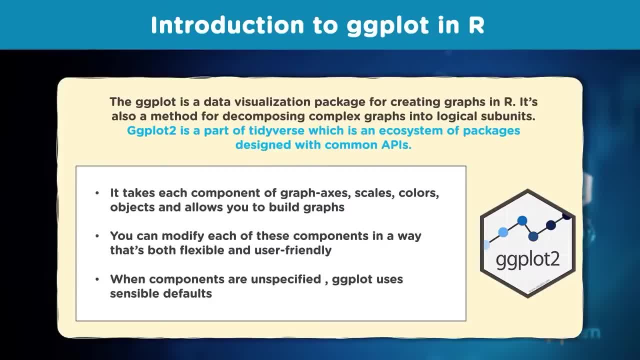 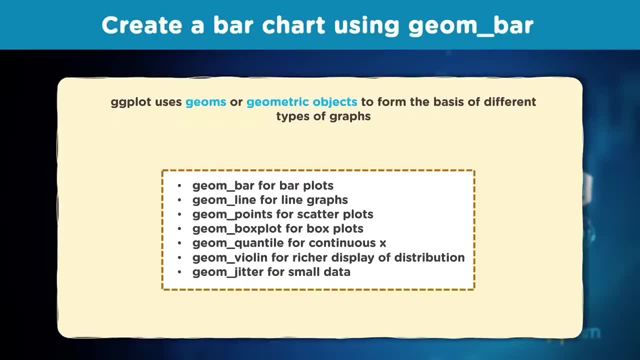 details for the components, then ggplot will use sensible defaults, and this basically makes it a powerful and a flexible tool. now here are different options when you use your ggplot, such as you can use geom, or what we call as geometry objects, to form the basis of different type. 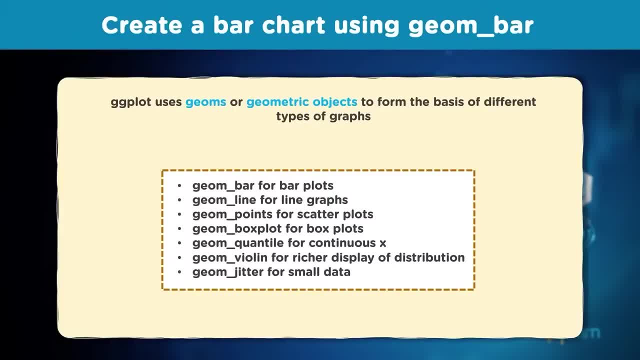 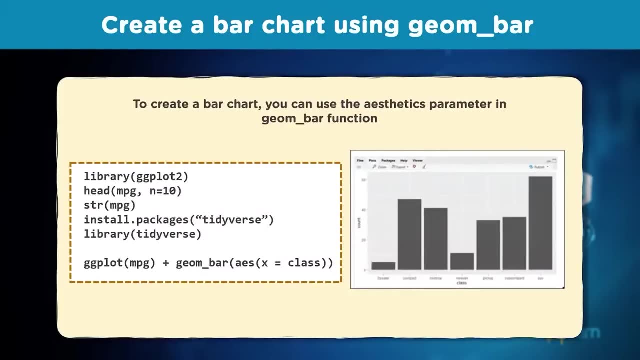 of graphs. for bar charts you have for line graphs, you have scatter plots, that is a underscore point. you have underscore box plot for box plots. you have quartile for continuous x, violin for richer display of distribution and jitter for small data. so here is some simple example where 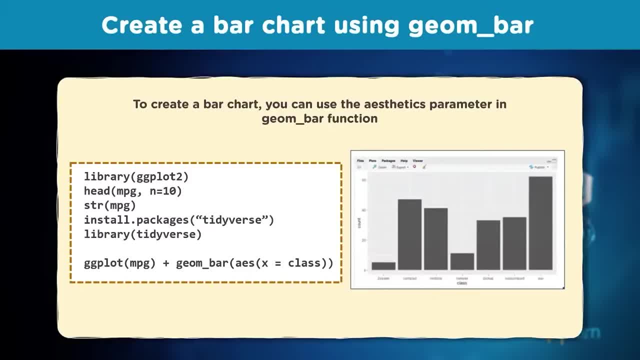 I would not go into too many details here, but you can just have a look at this one where we are using library function to get the ggplot to package. then, basically, we would want to look into the mileage data, we would want to look at the structure of it. 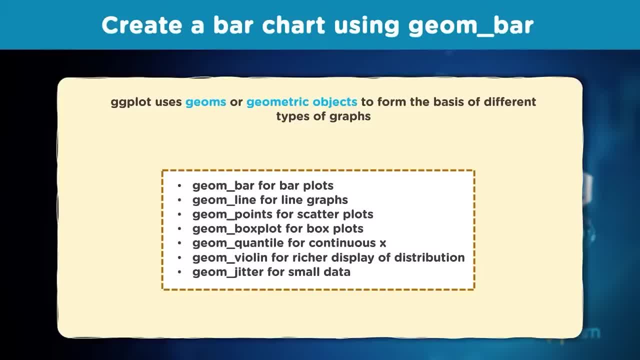 different options when you use your ggplot, such as you can use geom, or what we call as geometry objects to form the basis of different type of graphs. for bar charts you have. for line graphs, you have scatter plots. that is underscore point. you have underscore box plot. 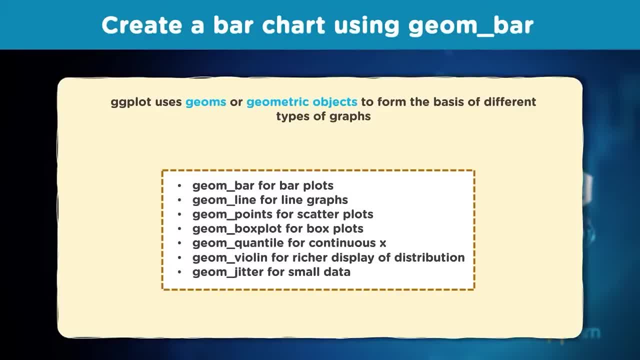 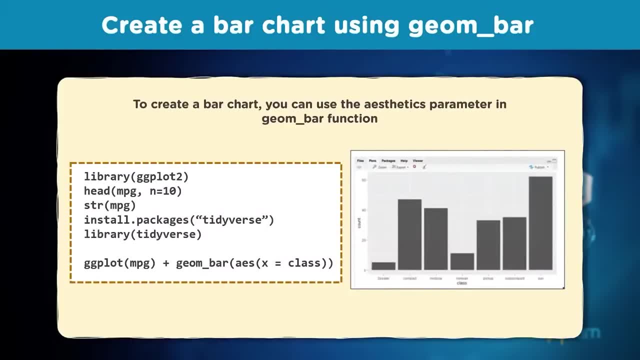 for box plots. you have quartile for continuous x, violin for richer display of distribution and jitter for small data. so here is some simple example where i would not go into too many details here, but you can just have a look at this one where we are using 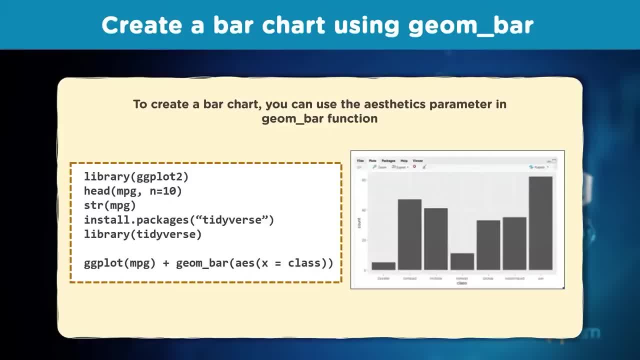 library function to get the ggplot2 package. then, basically, we would want to look into the mileage data, we would want to look at the structure of it and then we can basically get the tidyverse package. finally, we can create a bar chart using geom underscore bar. 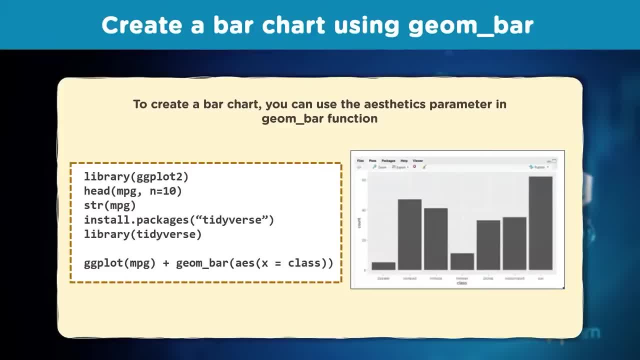 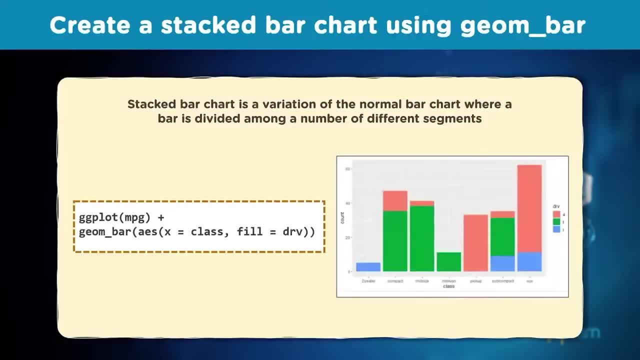 and we can basically also mention what would be in x axis. now you can also give different colors to basically add more meaning to your data. you could also go for stacked bar charts. so here we are actually telling ggplot to map the data in the drive column to fill. 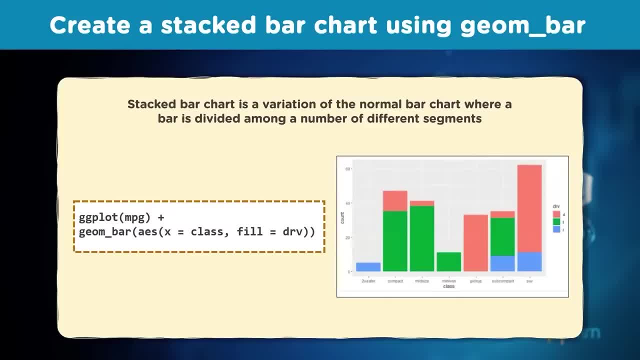 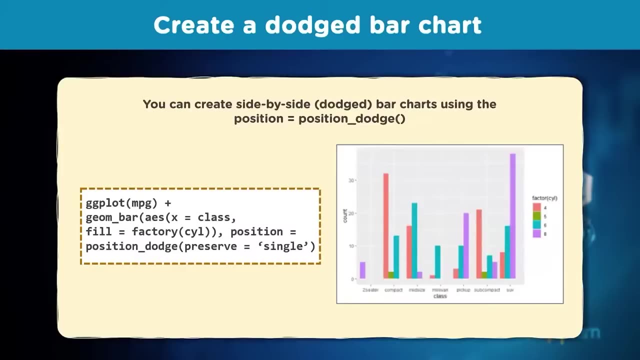 the aesthetic. so here i am giving aesthetic access class and i am saying what is the data we need to have? and then we are using geom underscore bar so you can also have dodged bar in your ggplot. that is not bar charts which are stacked, but 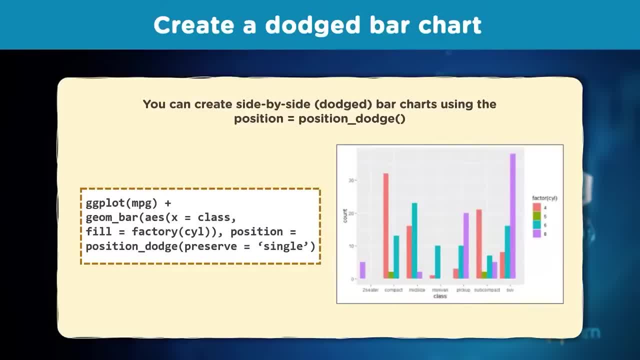 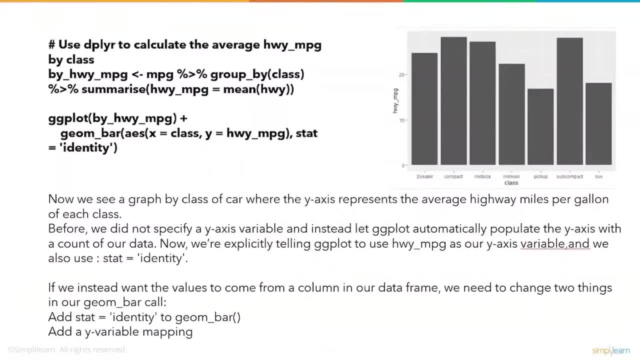 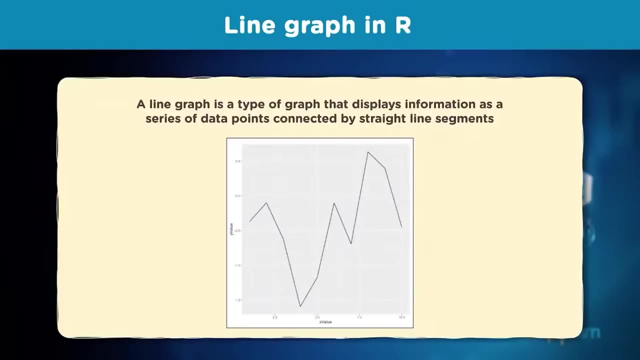 next to each other, and you can create that by using your position as position underscore dodge. okay, now you can obviously use your different packages, which are inbuilt, and you can create your bar charts, and you have other kind of graphs, such as line graph, which is basically. 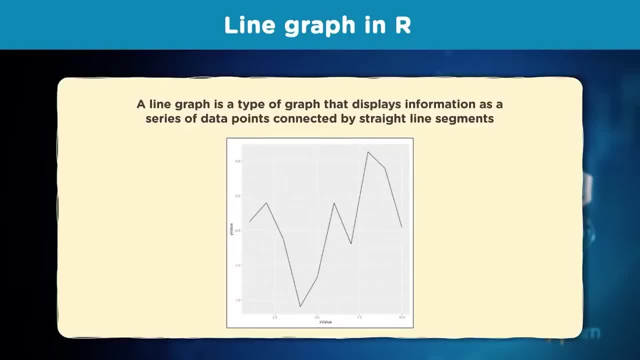 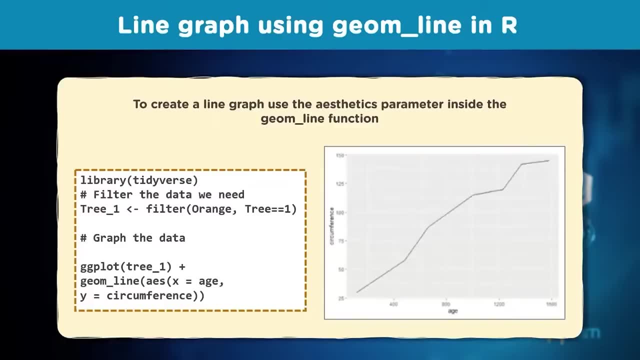 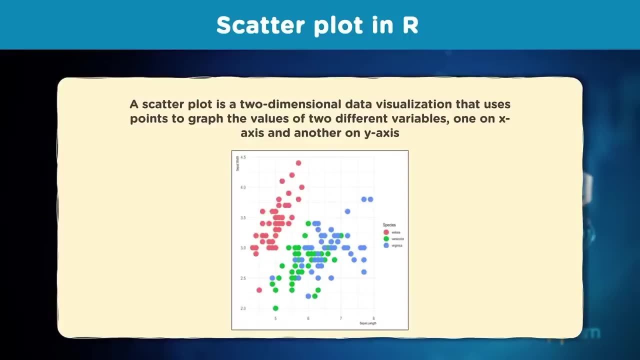 a type of graph that displays information as a series of data points connected by straight line segments such as this one, and for this one we are using, if you see, geom underscore line. now you can also create a scatter plot, which is a two dimensional data visualization that uses points. 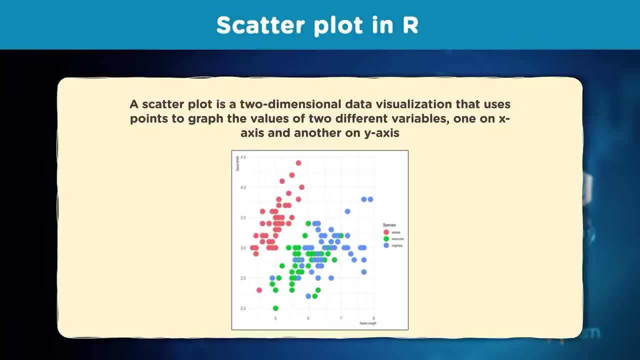 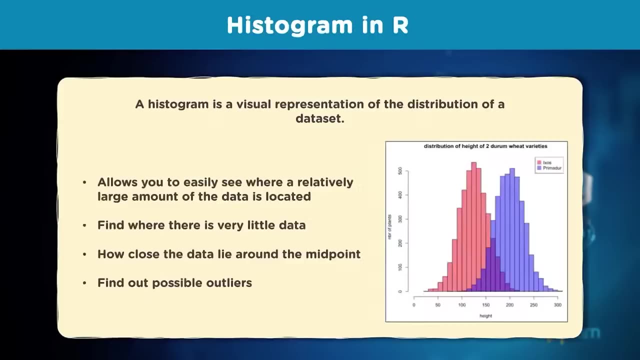 to graph the values of two different variables, one in x axis, one on y axis, like what we saw in base graphics, example, and they are mainly used if you would want to assess the relationship or lack of relationship between two variables, and you also have histogram, which i mentioned. 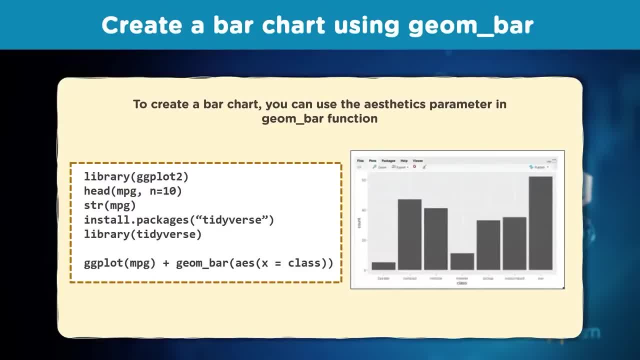 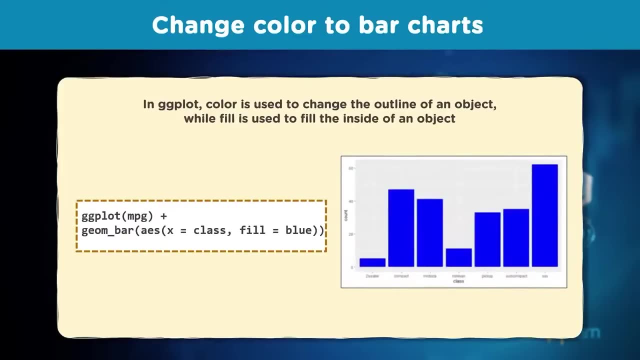 and then we can basically get the tidy verse package. finally, we can create a bar chart using geom underscore bar and we can basically also mention what would be in x axis. now you can also give different colors to basically add more meaning to your data. you could also go for stacked bar charts. 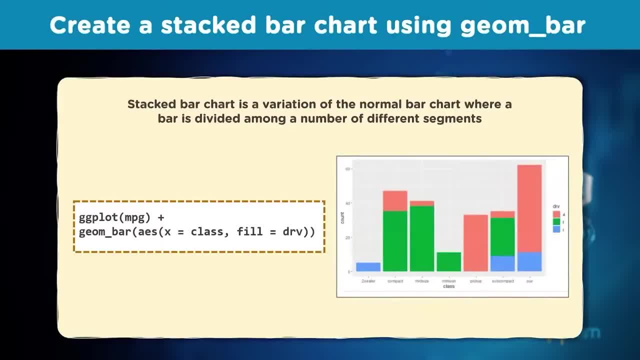 so here we are actually telling ggplot to map the data in the drive column to fill the aesthetic. so here I am giving aesthetic access class and I am saying what is the data we need to have, and then we are using geom underscore bar. so you can also. 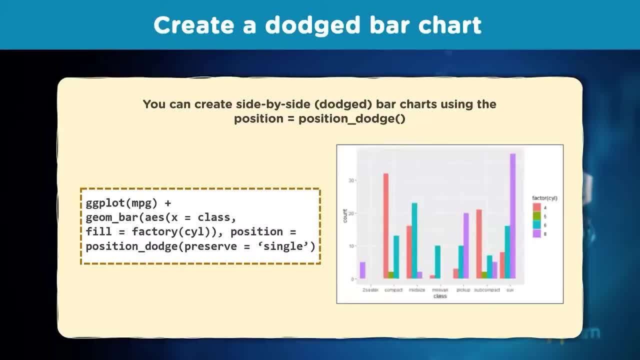 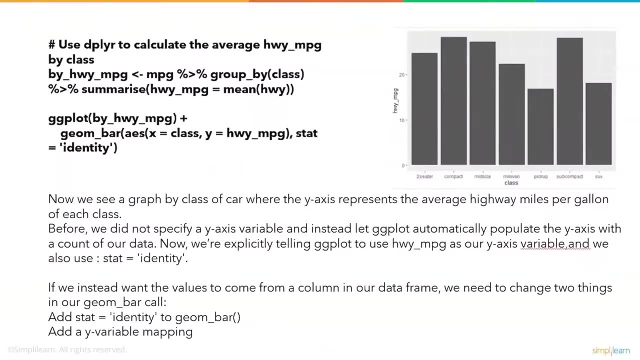 have dodged bar in your ggplot, that is, not bar charts which are stacked but next to each other, and you can create that by using your position as position underscore dodge. now you can obviously use your different packages, which are inbuilt, and you can create your bar charts. 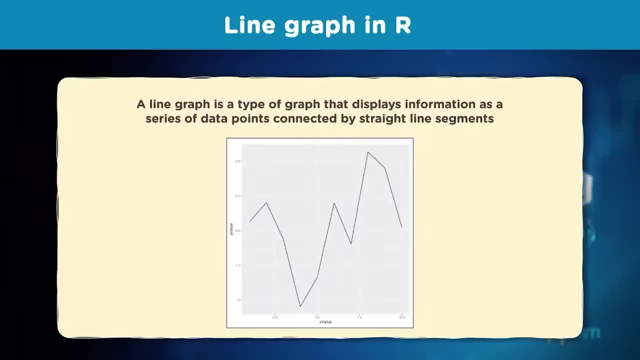 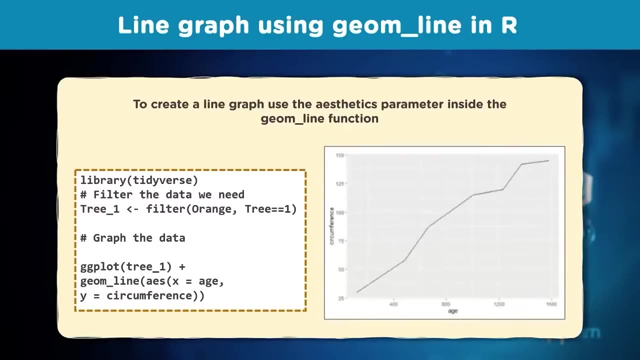 and you have other kind of graphs, such as line graph, which is basically a type of graph that displays information as a series of data points connected by straight line segments such as this one, and for this one we are using, if you see, geom underscore line. now you can also 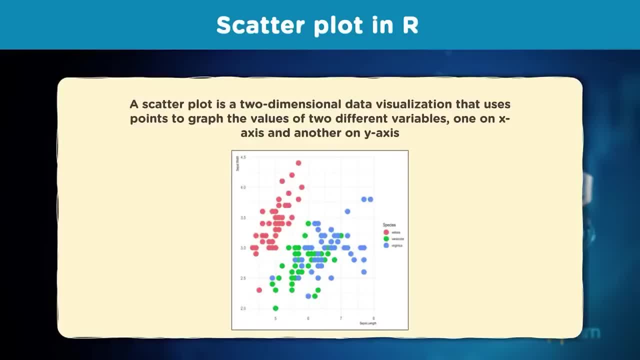 create a scatter plot, which is a two dimensional data visualization that uses points to graph the values of two different variables- one on x axis, one on y axis, like what we saw in base graphics, example, and they are mainly used if you would want to assess the relationship. 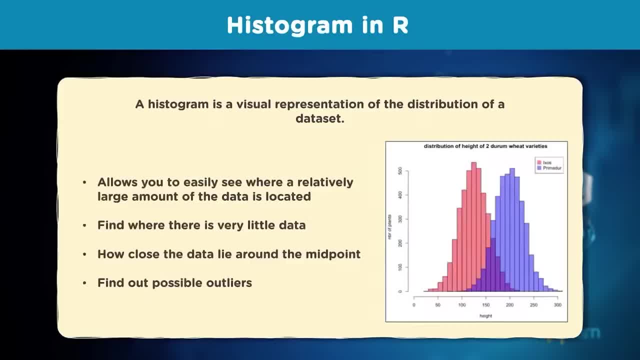 or lack of relationship between two variables. and you also have histogram, which I mentioned is mainly to look at the distribution of a data, to look at the central tendency of the data, basically looking at your large amount of data or, for a single variable, you would be interested in saying where is? 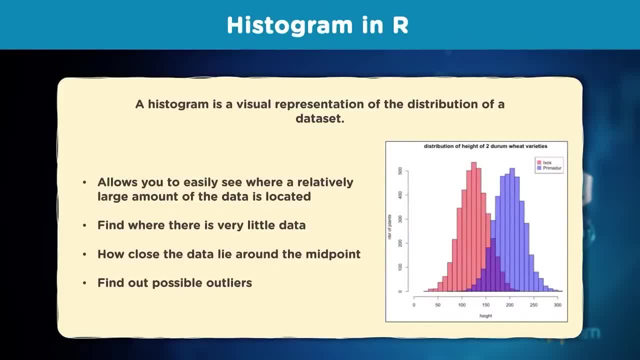 is mainly to look at the distribution of a data, to look at the central tendency of the data. basically looking at your large amount of data or, for a single variable, you would be interested in saying where is more data found in terms of frequency? where is lesser data found in the graph? 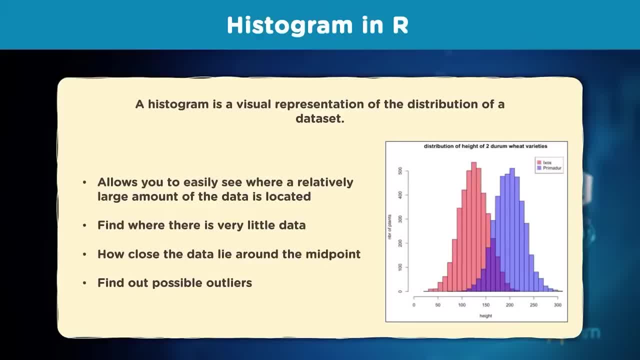 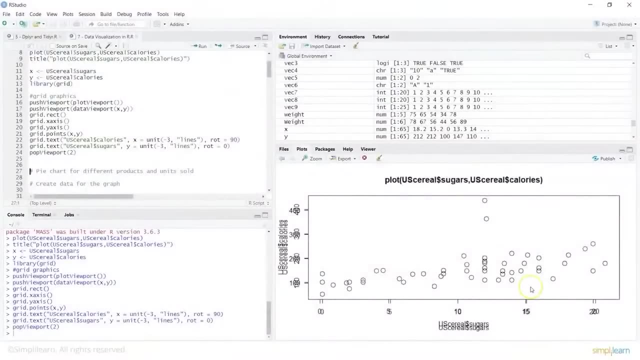 how close the data is towards its mid point, or what we call as mean median mode. so you can use histogram where you can categorize the data in what we call as bins. so these are some basics on different kind of graphs. now we can look at some examples and see. 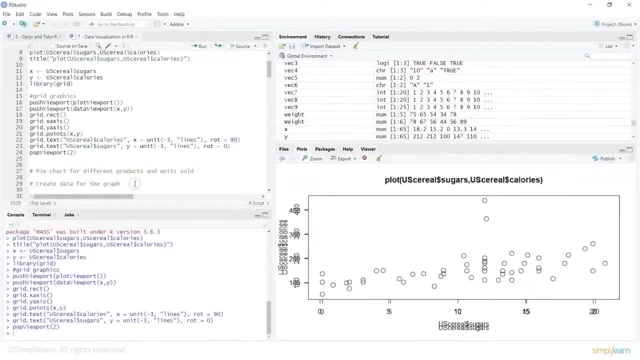 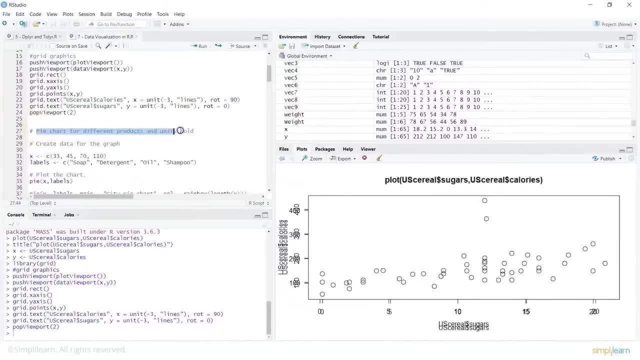 how that works. so what we were seeing is some quick examples of base graphics or grid graphics. now here lets do an example of pi chart for different products and units sold. so you want to create a graph for this. first lets create a vector and pass in the value here. 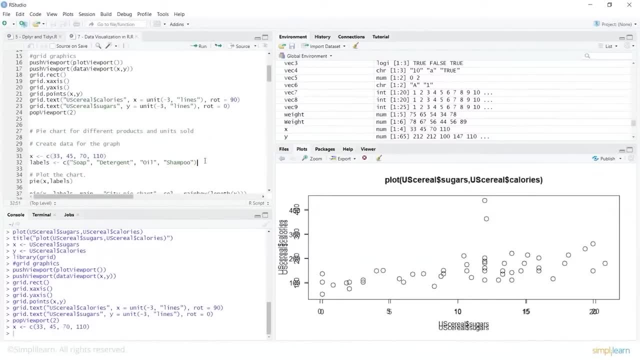 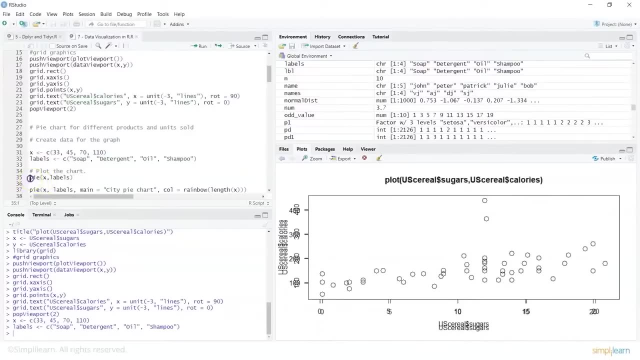 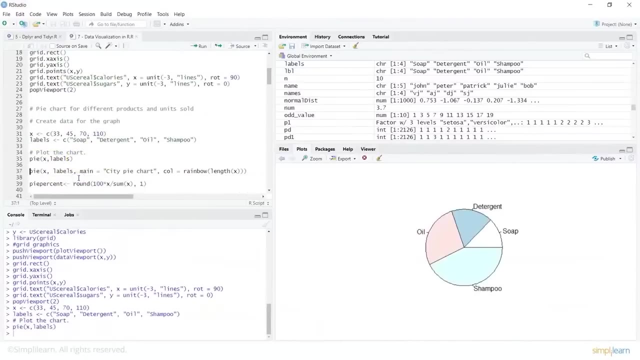 now i can also create labels which i would want to assign to these values and then, basically, i can plot the chart by saying pi. so thats the kind of chart which i would want to create and i would say the data would be x and labels. so lets. 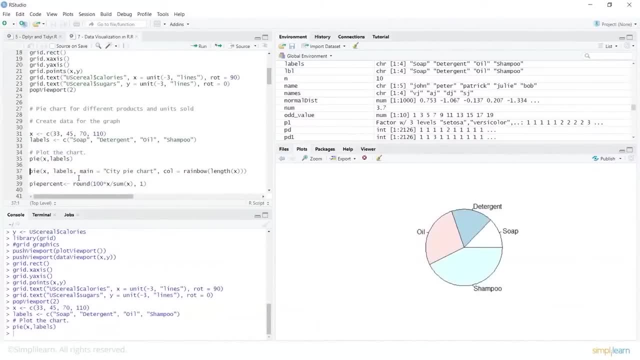 do this and that shows me a simple pi chart. now i can also give main details here. so instead of just doing a pi x comma labels, i can say what is the main and then what kind of coloring it should follow. so this is the way you can create a simple. 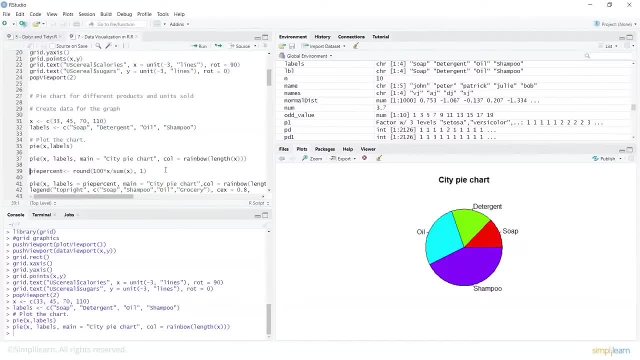 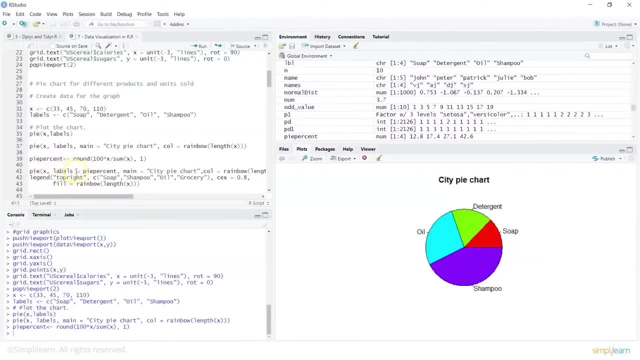 plot, now i can also find out what is the percentage. and then, basically, i would be interested in plotting the pi chart which takes x, which takes the labels, which will be the percentage which we are calculating here by doing a round function, and then you can basically give details to your 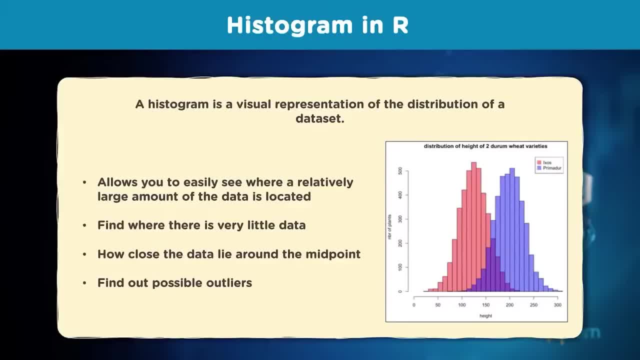 more data found in terms of frequency. where is lesser data found in the graph? how close the data is towards its mid point, or what we call as mean median mode? so you can use histogram where you can categorize the data in what we call as bins. so these are: 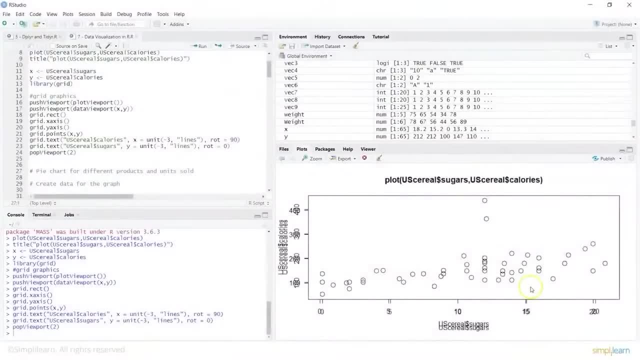 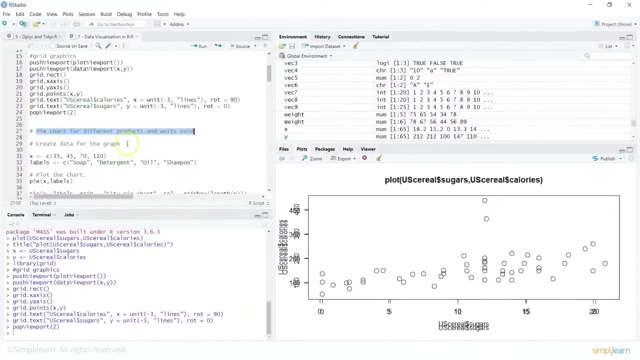 some basics on different kind of graphs. now we can look at some examples and see how that works. so what we were seeing is some quick examples of base graphics or grid graphics. now, here lets do an example of pie chart for different products and units sold. so you want to create 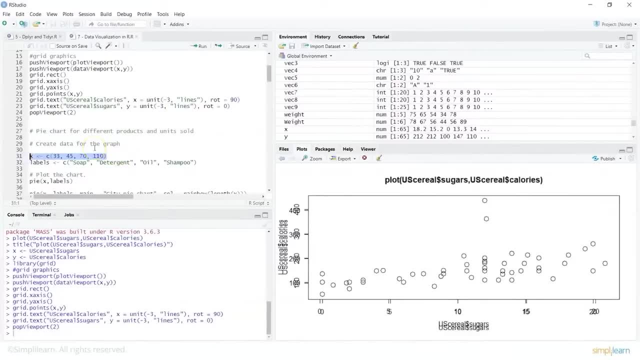 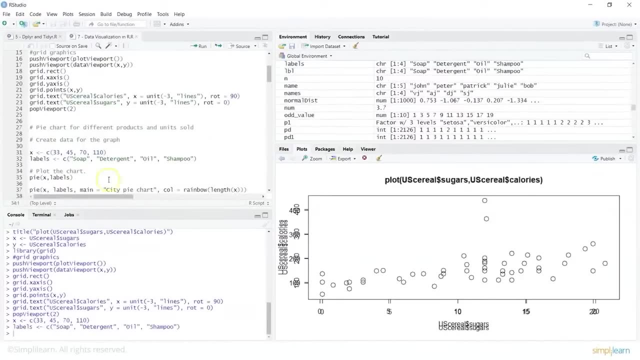 a graph for this. first, lets create a vector and pass in the value here. now I can also create labels which I would want to assign to these values and then basically, I can plot the chart by saying pie. so that's the kind of chart which I would want to create, and 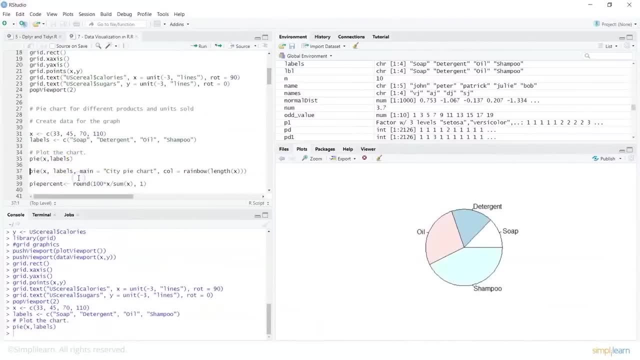 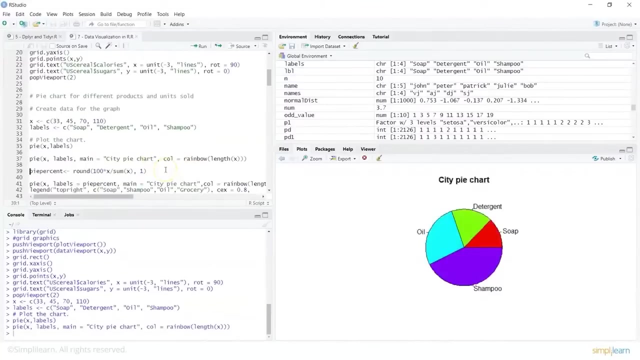 I would say the data would be x and labels. so lets do this. and that shows me a simple pie chart. now I can also give main details here. so instead of just doing a pie x comma labels, I can say what is the main and then what kind of coloring it should follow. 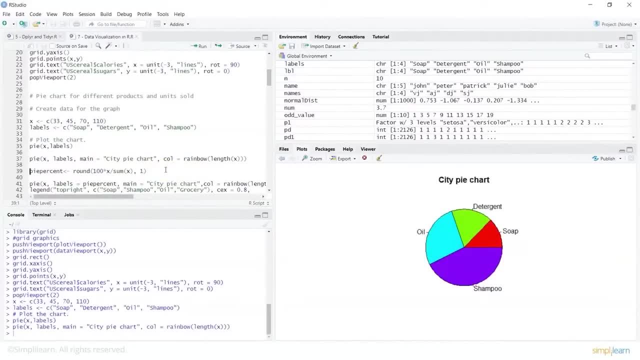 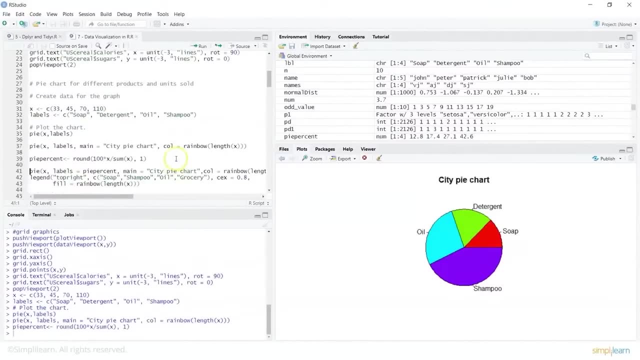 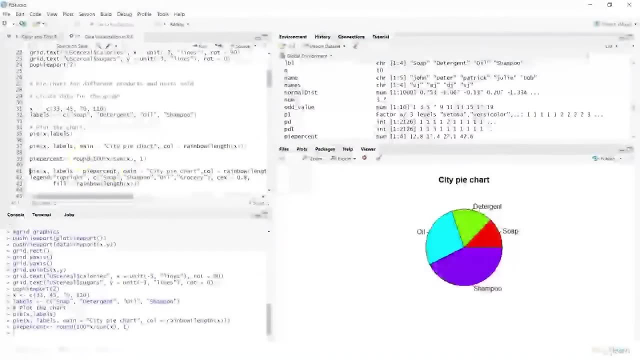 so this is the way you can create a simple plot. now I can also find out what is the percentage. and then, basically, I would be interested in plotting the pie chart which takes x, which takes the labels, which will be the percentage which we are calculating here by doing a. 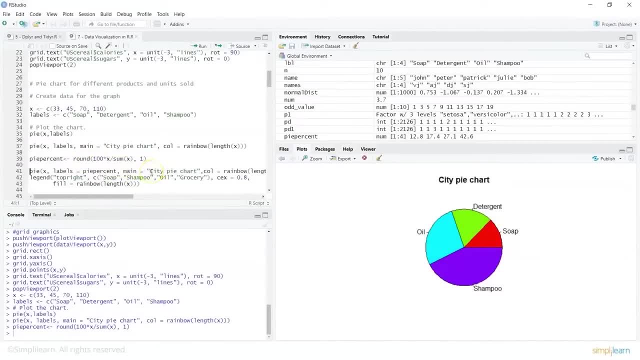 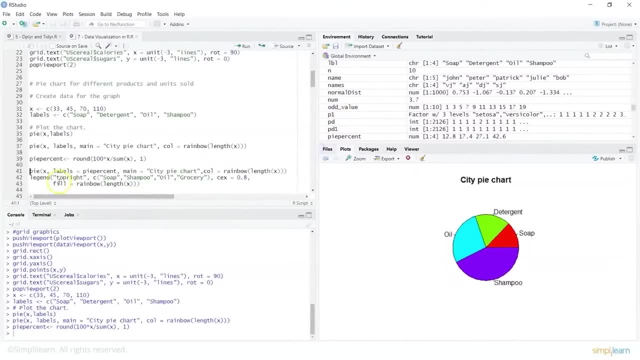 round function and then you can basically give details to your graph. you can say what color it follows, you can basically look at the legend, where it needs to be in your chart- what are the values- and then basically fill up the colors. so lets run this one and that shows me. 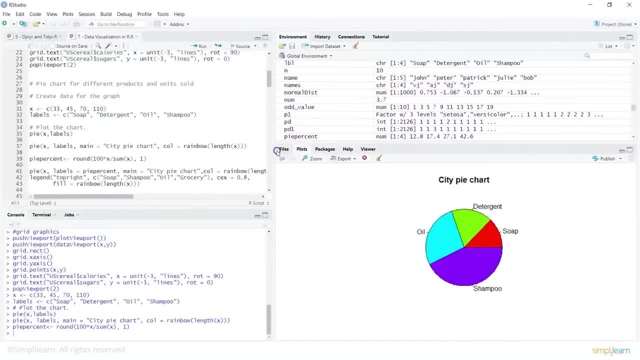 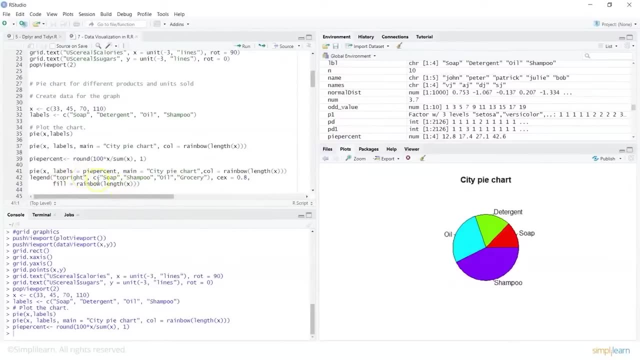 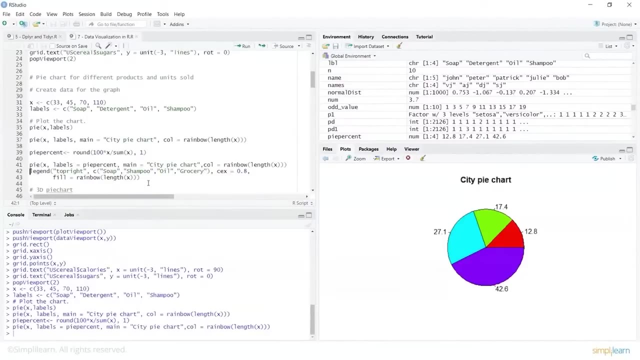 graph. you can say what color it follows. you can basically look at the legend, where it needs to be in your chart- what are the values, and then basically fill up the colors. so lets run this one and that shows me the percentage which was calculated and it gives me the details. 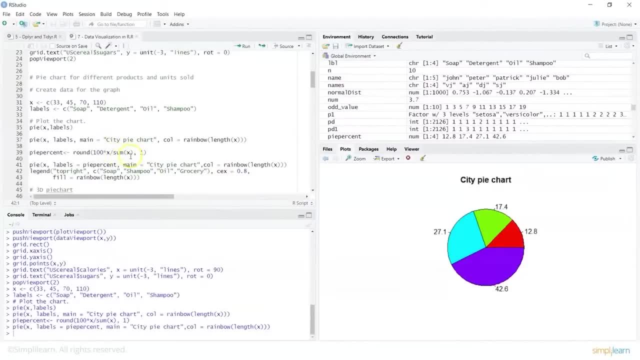 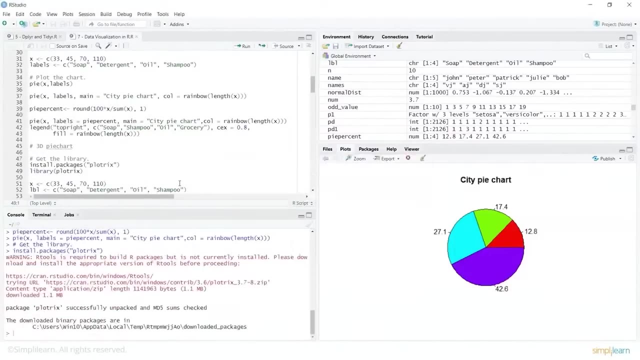 the percentage which was calculated and it gives me the details and we can always have a look at our plot. now, if you would want to go for a 3D pie chart, then you can get the package which is plotrix. lets use that by calling in: 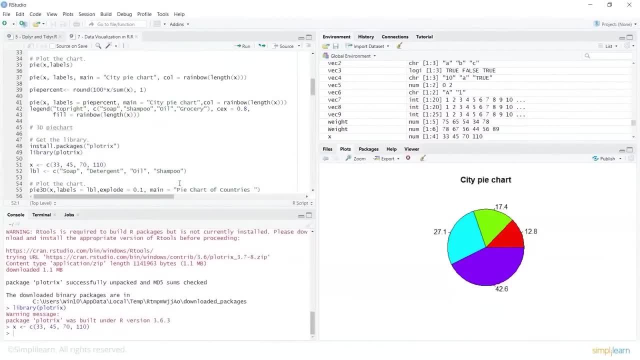 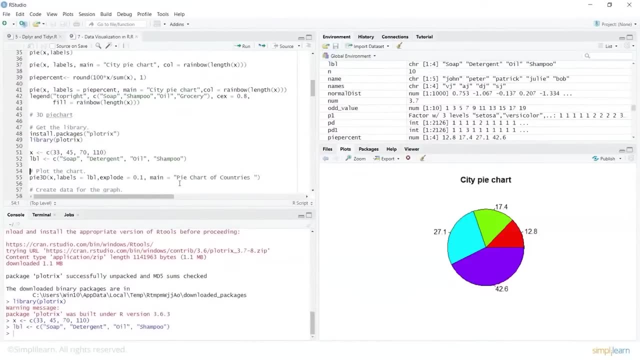 the library function lets pass in some data to x and lets give some values or labels which will make more meaning to the data, and then lets plot the 3D graph. so I am saying pie 3D here, where I am using x and labels. then I am basically doing an explode. 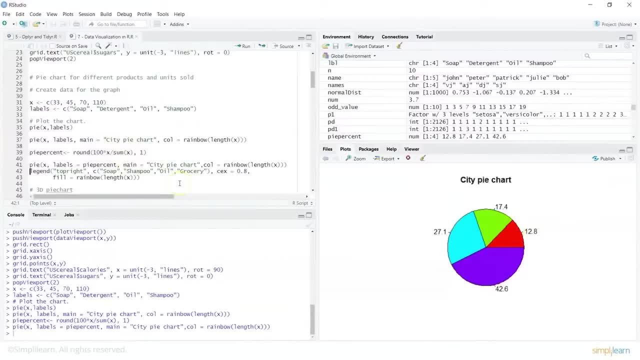 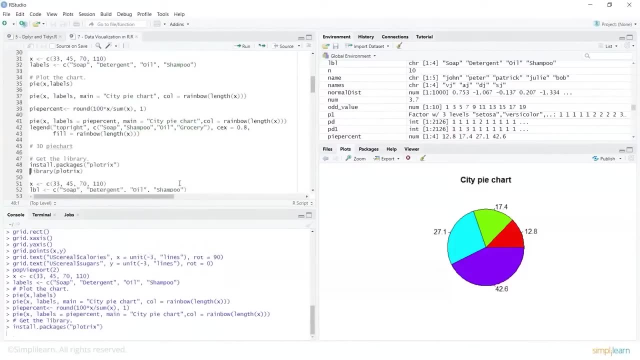 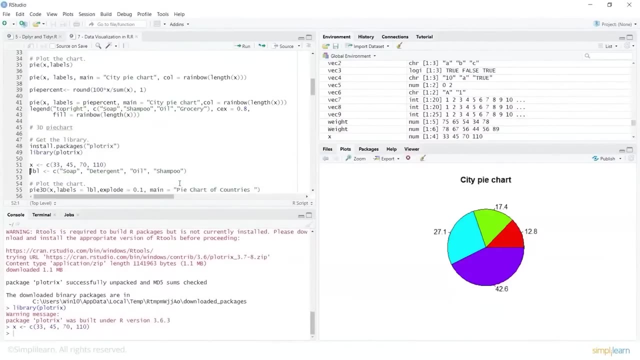 and we can always have a look at our plot. now, if you would want to go for a 3d pi chart, then you can get the package which is plotrix. lets use that by calling in the library function. lets pass in some data to x and lets give some values. 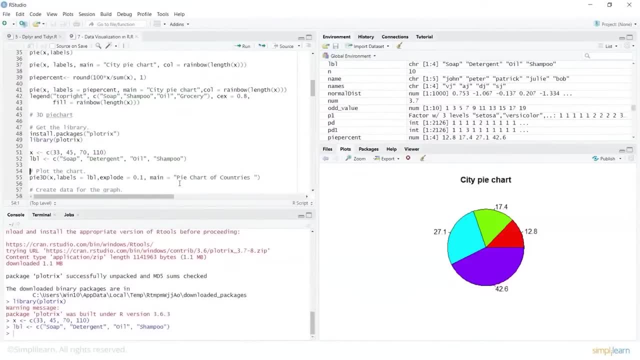 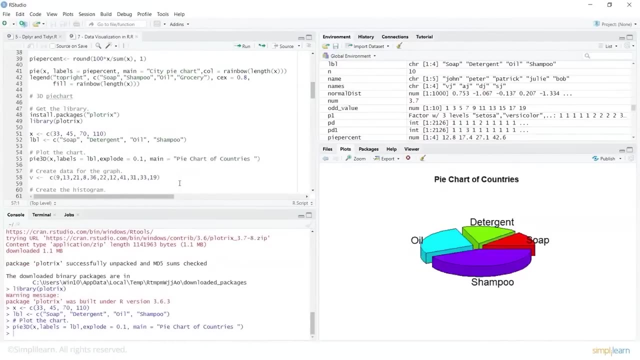 or labels, which will make more meaning to the data. and then lets plot the 3d graph. so i am saying pi 3d here, where i am using x and labels. then i am basically doing an explode which will basically control how your graph looks like and basically, 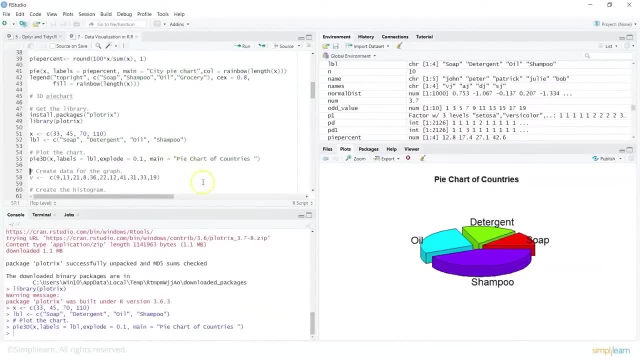 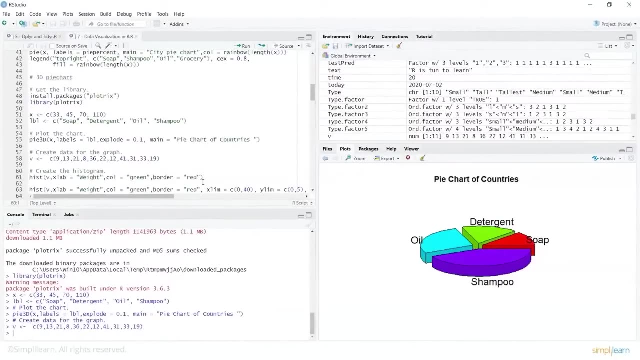 give the values. so it also takes the title when you say main and pi chart of countries. now lets create data for graph. so again we are having a variable here. we are using the c function creating a vector, and then lets create a histogram for this one, where i would say: 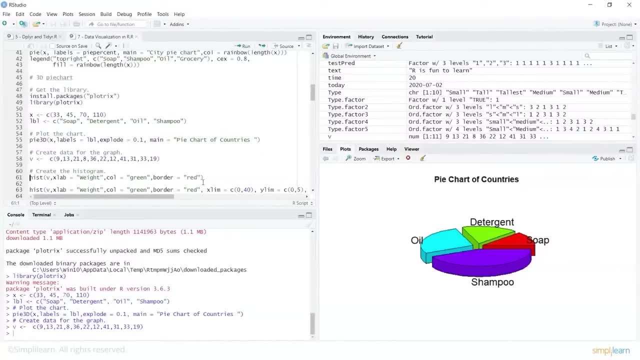 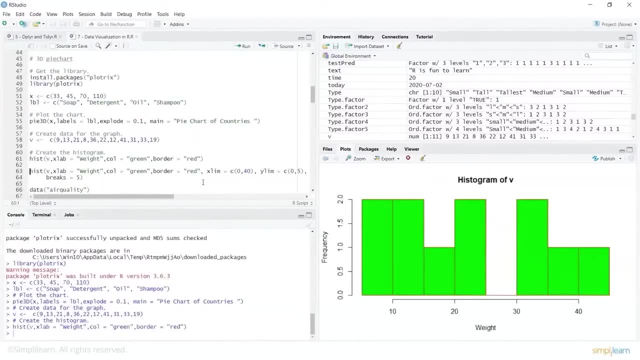 xlab. what would be your data around x axis? what is the color, what is the border? and here i am creating a simple histogram which, as i discussed earlier, will always show your values on the x axis, and y axis is more of frequency, and then you can look. 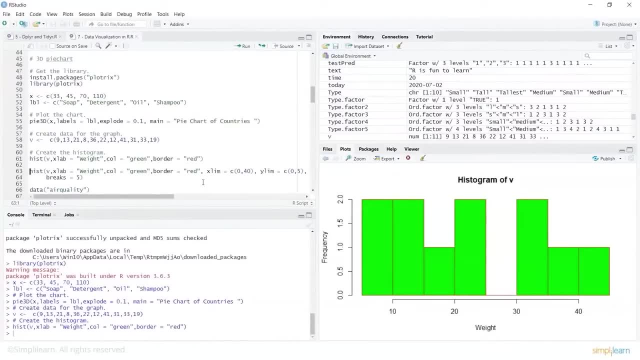 at the set of values and what is their frequency, and we can basically use this histogram for exploratory data analysis. look at the data, try to understand what is the central tendency of your data values. now we can also give some limits by using the xlim and ylim and then 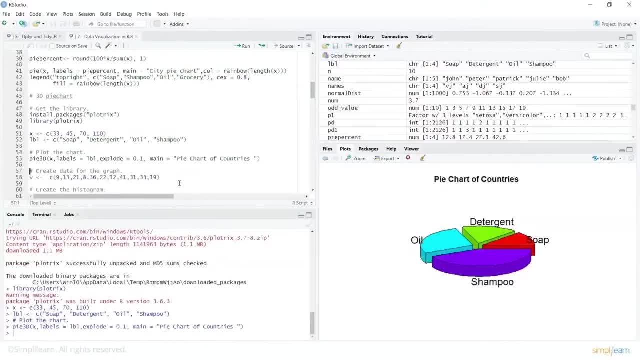 which will basically control how your graph looks like and basically give the values. so it also takes the title when you say main and pie chart of countries. now lets create data for graph. so again we are having a variable here. we are using the c function, creating a vector and 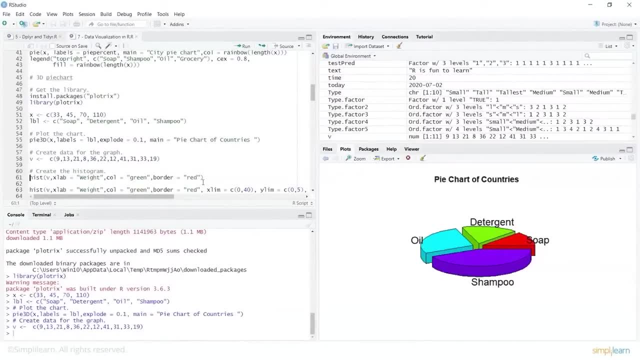 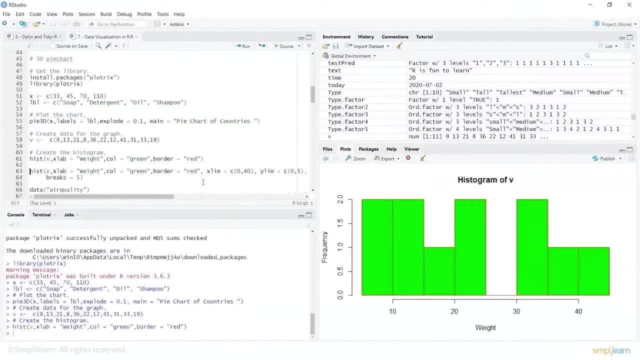 then lets create a histogram for this one, where I would say: x lab. what would be your data around x axis? what is the colour, what is the border? and here I am creating a simple histogram which, as I discussed earlier, will always show your values on the x axis and y axis is more. 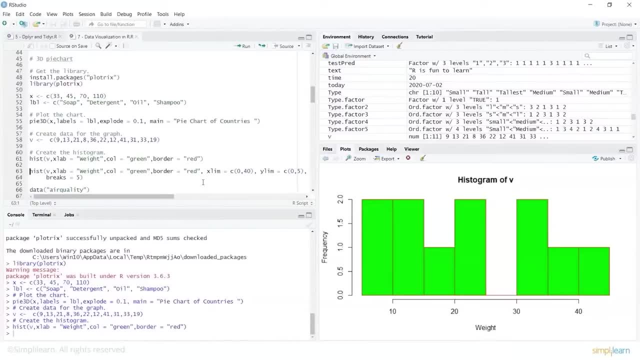 of frequency and then you can look at the set of values and what is their frequency, and we can basically use this histogram for exploratory data analysis. look at the data, try to understand what is the central tendency of your data values. now we can also give some limits by using the 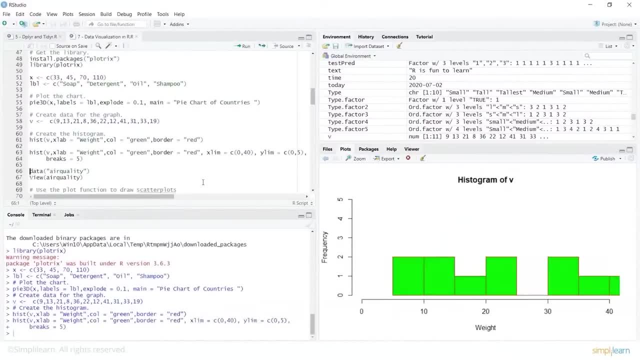 x limb and y limb, and then I can also specify what is the limit. so we have given some values here wherein we have said: your x limit is 0 to 40 and y limit is 0 to 5. now, if you compare this with the previous, 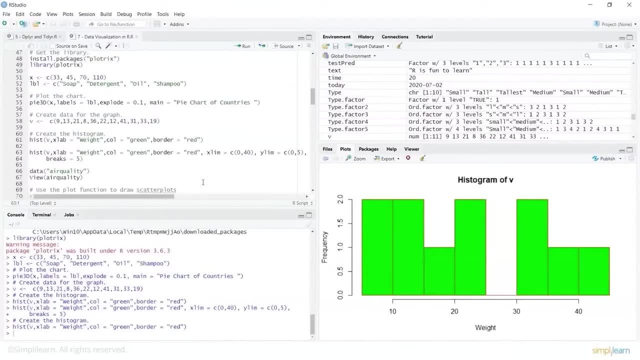 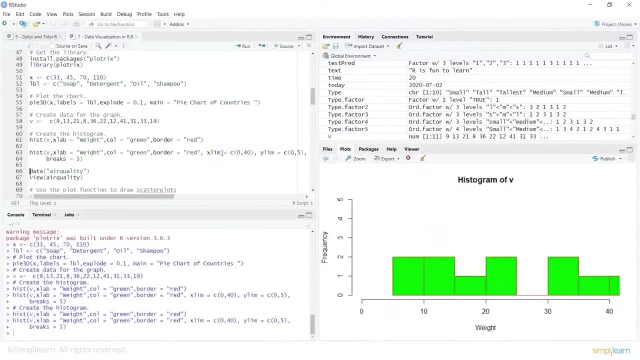 one which we had created. this one, based on the frequency, had taken the limits, but we can assign limits explicitly by giving this and then create a histogram which makes more meaning. now let's take another data set, that is air quality. let's view this to see. what does that data contain? 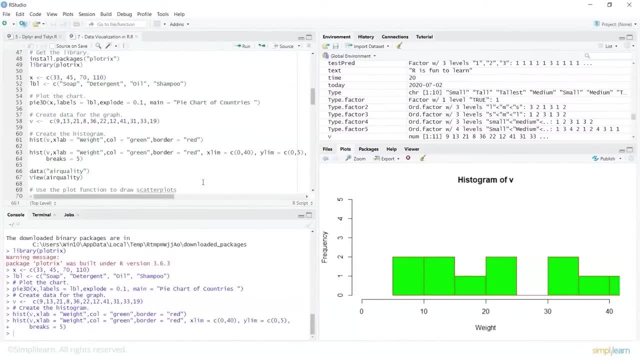 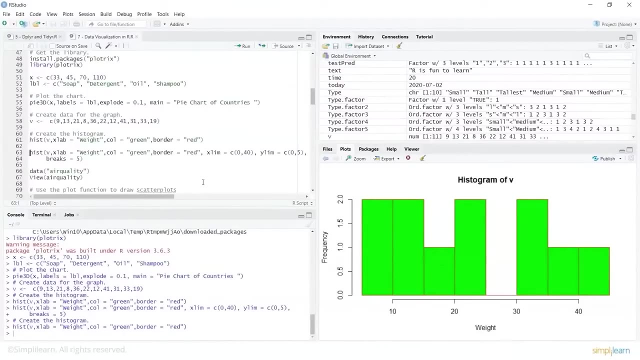 i can also specify what is the limit. so we have given some values here wherein we have said: your xlim is 0 to 40 and ylim is 0 to 5. now, if you compare this with the previous one which we had created- this one based on the frequency- 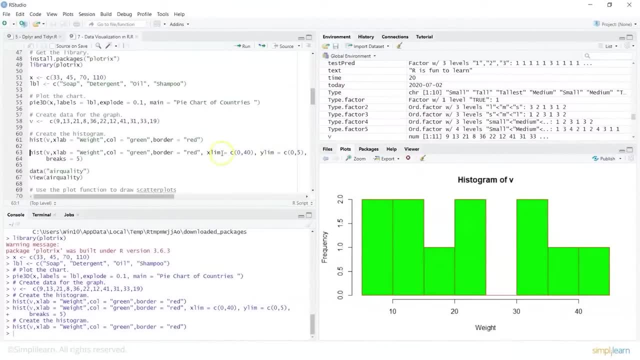 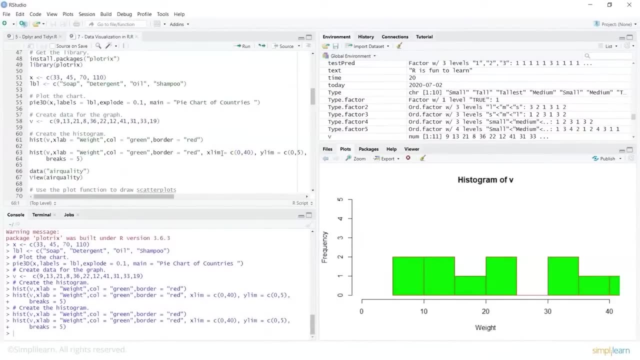 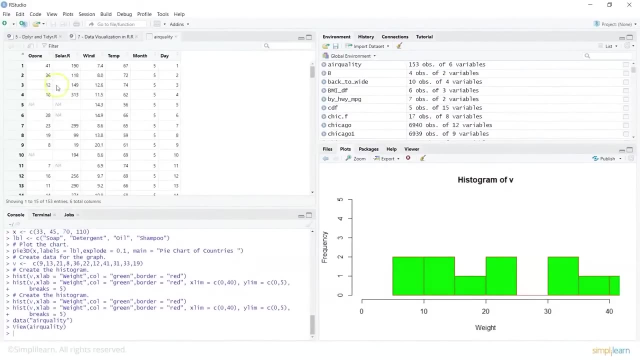 had taken the limits. but we can assign limits explicitly by giving this and then create a histogram which makes more meaning. now let's take another data set, that is air quality. let's view this to see. what does that data contain? so you have ozone, solar, wind, temperature month. 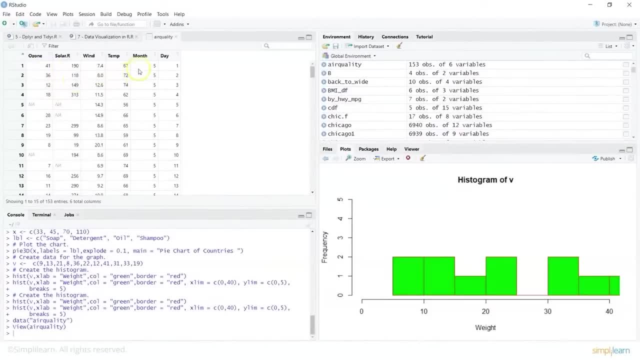 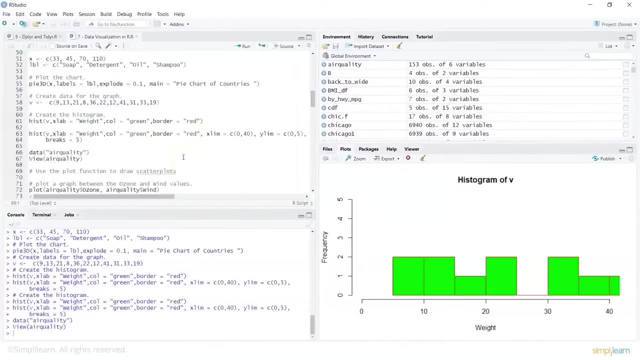 so you have ozone, solar, wind, temperature, month and the day. so this is the kind of information we have in the air quality. now let's use the plot function to draw a scatter plot where, as I mentioned, you would be interested in analyzing variables and see what is the relationship between them. 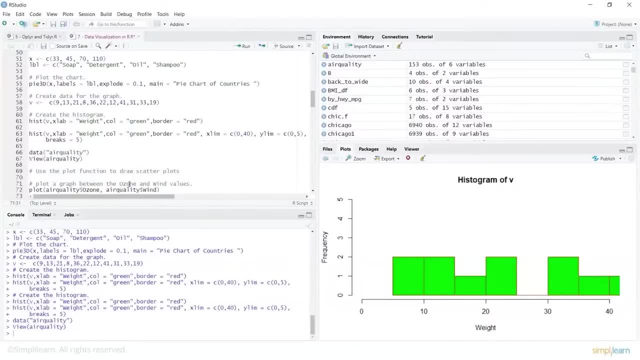 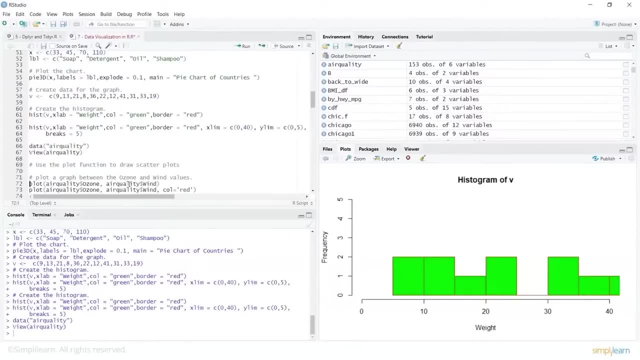 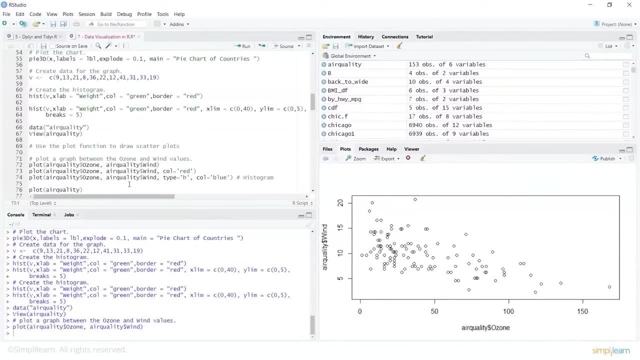 so to plot a graph between ozone and wind values. so we will say plot, we will say the data, which is air quality. from that I would be interested in the ozone column or ozone field and the wind field. I can create a plot based on this. now I can also be saying: 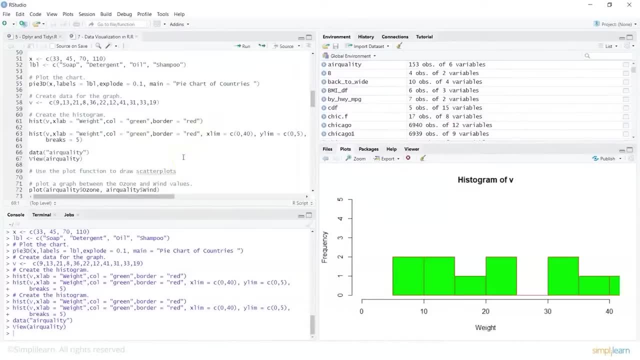 and the day. so this is the kind of information we have in the air quality. now let's use the plot function to draw a scatter plot where, as i mentioned, you would be interested in analyzing variables and see what is the relationship between them. so to plot a graph between 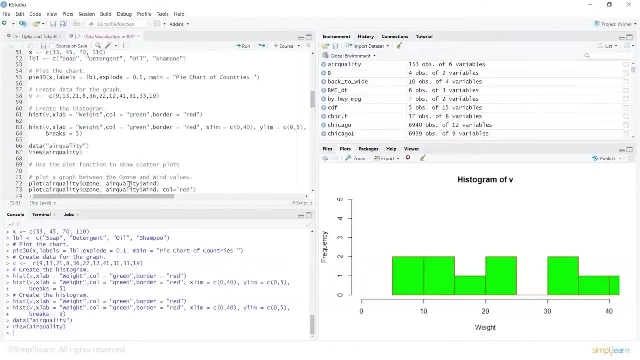 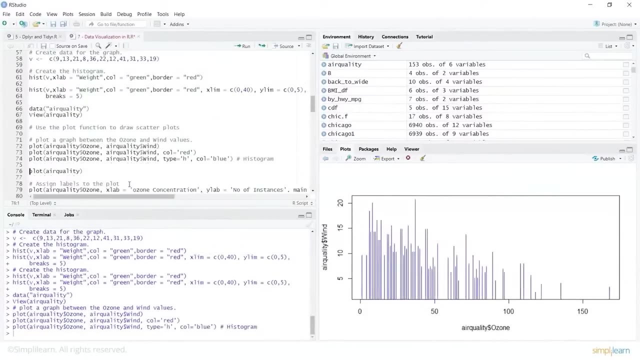 ozone and wind values. so we will say plot, we will say the data, which is air quality. from that i would be interested in the ozone column or ozone field and the wind field. i can create a plot based on this. now i can also be saying what should be the color, what is the 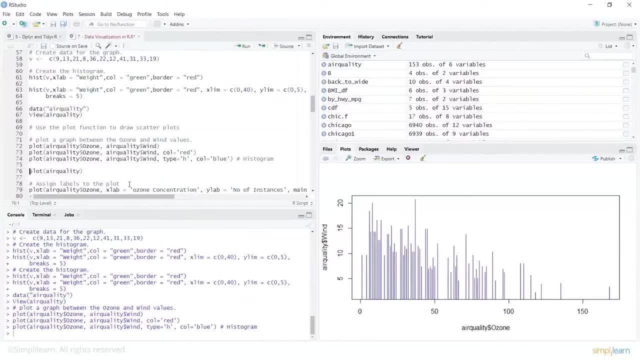 type of the data which you would want to create and you can look at the information so you can create a histogram, you can create a scatter plot to basically understand the data better and then infer some information from that data. so let's take the air quality data set itself without 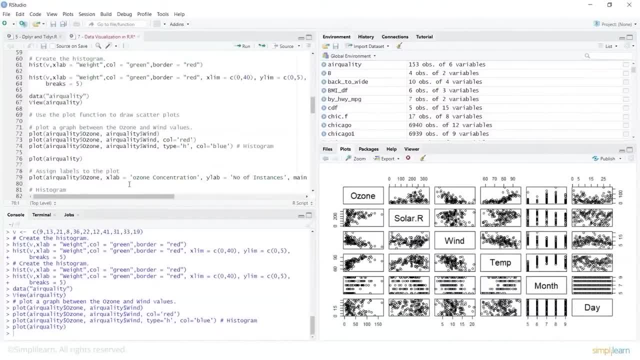 specifying any particular column and you can create a plot which shows me all the different values which you have in the data and it basically shows you the difference. this is more of an example, like what we did for chick weight, where we did a base graphics. now you can assign layers. 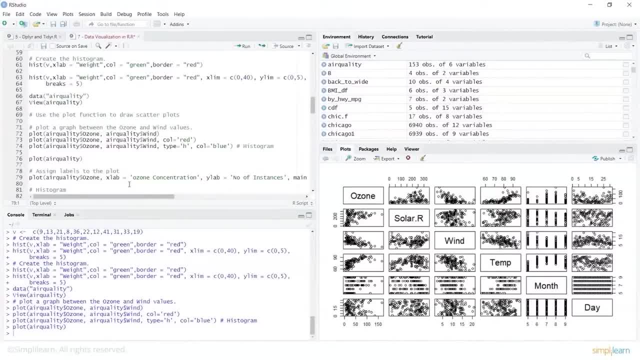 labels to the plot. so that is when you are creating a plot. you can say air quality, you will say ozone and then that's your ozone concentration. you have your y lab, which is the number of instances you have. what is the title? ozone levels in new york city. what is the color? 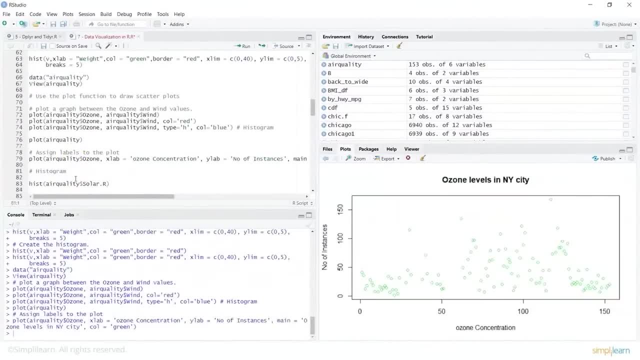 so these are the details, what we have given with our plot function, and let's look at the data. so it just tells me that this is the ozone concentration, the number of instances, what you have, and you are looking at the data now we could also create a histogram. 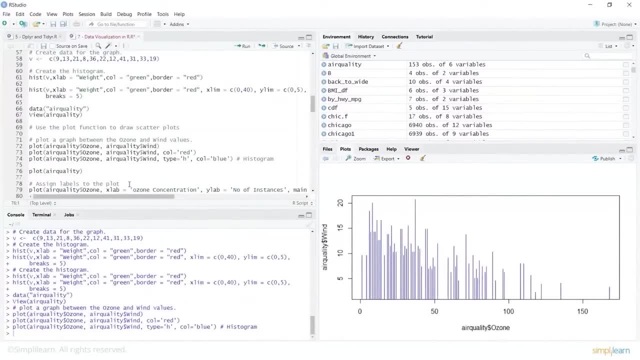 what should be the color, what is the type of the data which you would want to create and you can look at the information. so you can create a histogram, you can create a scatter plot to basically understand the data better and then infer some information from that data. so let's take the 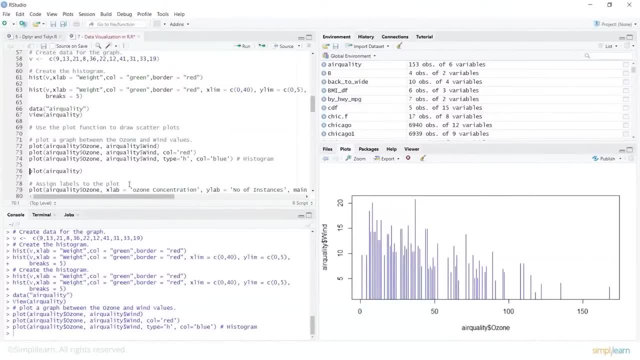 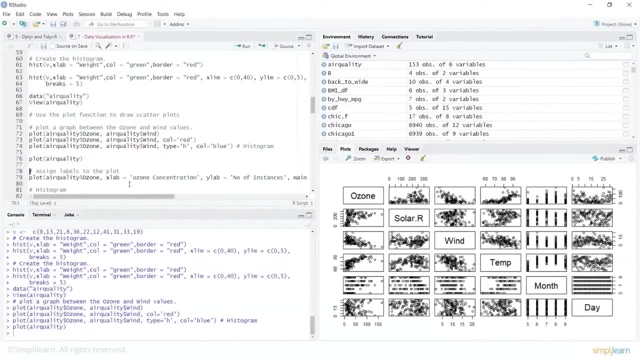 air quality data set itself without specifying any particular column, and you can create a plot which shows me all the different values which you have in the data and it basically shows you the difference. this is more of an example, like what we did for chick weight, where we did a 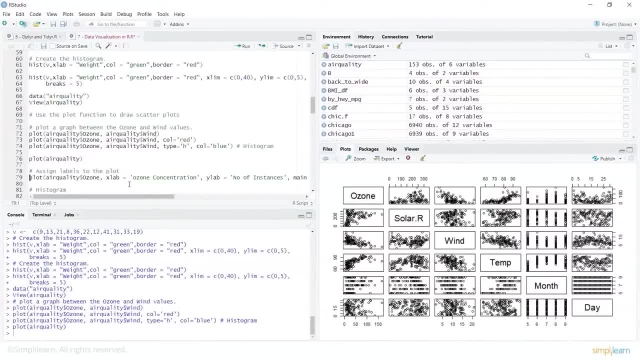 base graphics. now you can assign labels to the plot. so that is when you are creating a plot. you can say air quality, you will say ozone and then that's your ozone concentration. you have your y lab, which is the number of instances you have. what is the title? ozone levels. 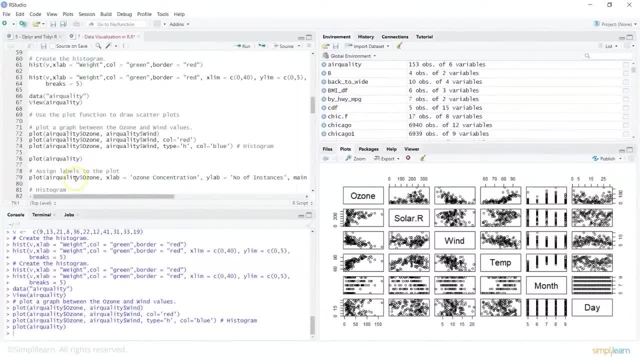 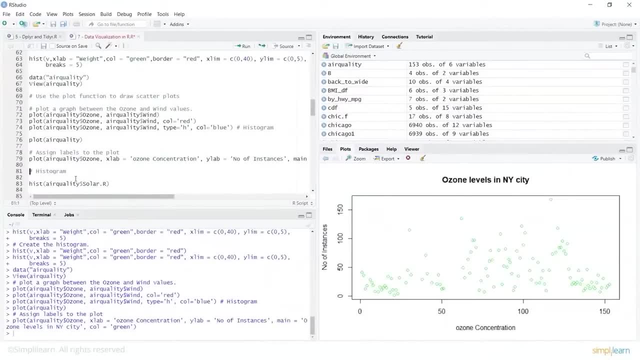 in New York City. what is the color? so these are the details, what we have given with our plot function, and let's look at the data. so it just tells me that this is the ozone concentration, the number of instances, what you have, and you are looking at the 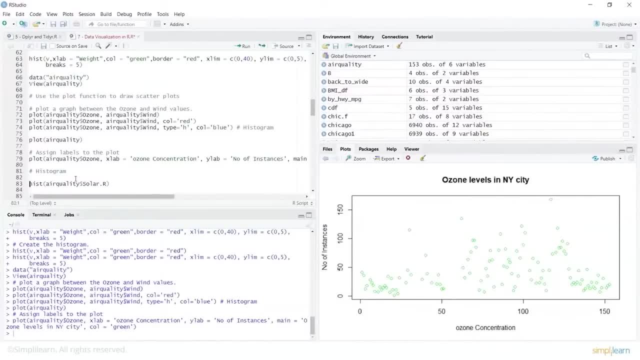 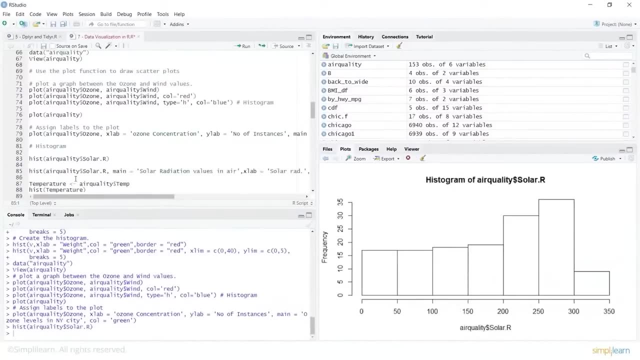 data. now we could also create a histogram by picking up a particular column that is such as solar, from your air quality and that basically shows me the frequency of solar values, and we can then try to find out what is the mid, what is the mean, what is the standard. 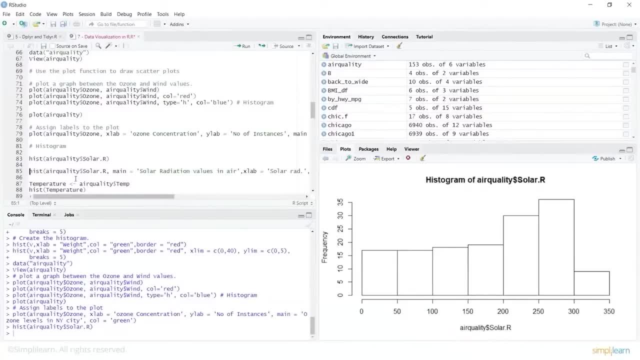 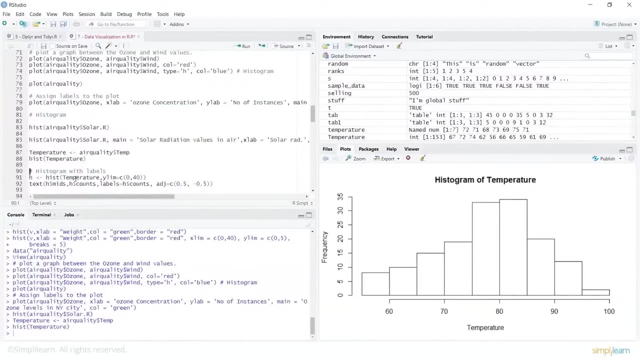 deviation and so on. you can also look at your histogram and try to understand if it is left skewed and right skewed. so we can do that now here. let's get the temperature out from this particular data set, let's create a histogram on temperature and that basically shows me. 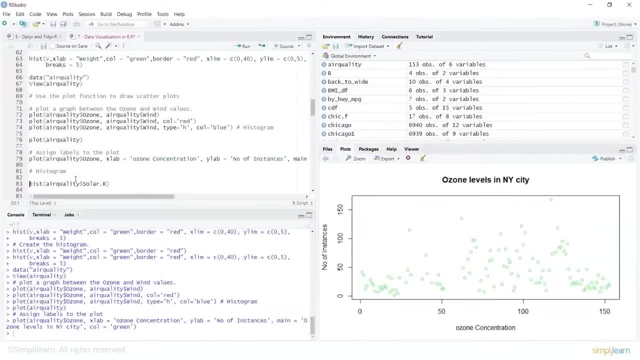 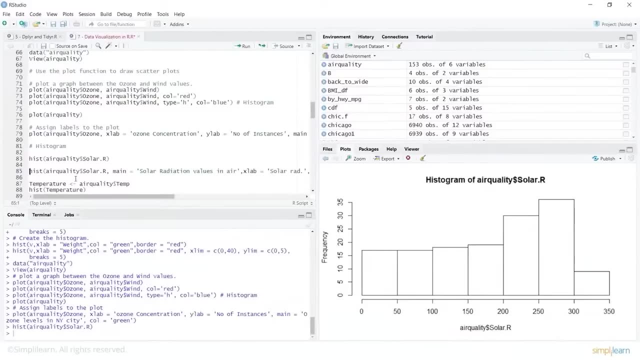 by picking up a particular column that is such as solar from your air quality and that basically shows me the frequency of solar values, and we can then try to find out what is the mid, what is the mean, what is the standard deviation, and so on. you can also look. 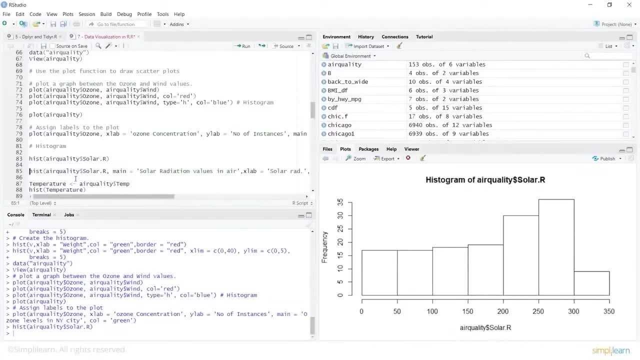 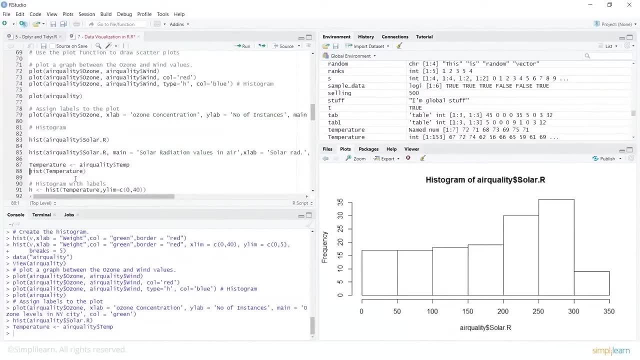 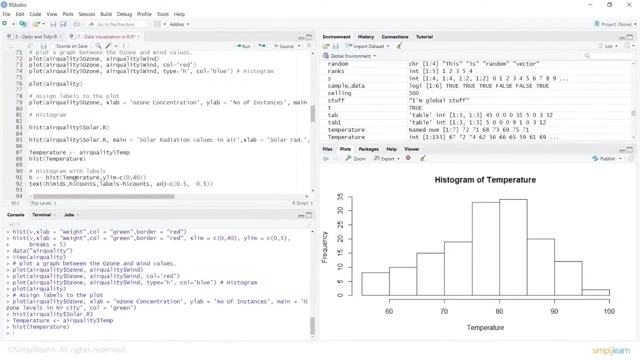 at your histogram and try to understand if it is left skewed and right skewed. so we can do that now here. let's get the temperature out from this particular data set, let's create a histogram on temperature and that basically shows me the frequency of the temperature values and 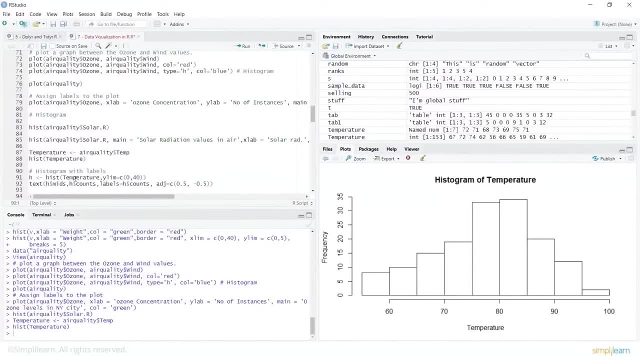 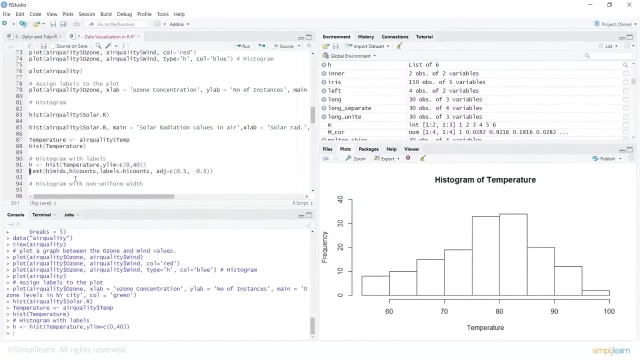 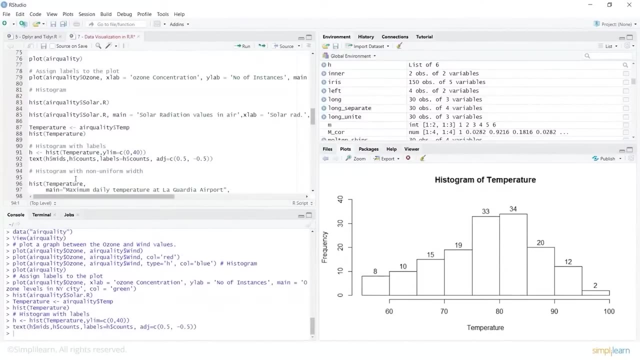 what values have the most frequency or most occurrence. now you can create a histogram with labels, so let's do that with the limit, and then let's also use text to basically give in the values, which also takes the values, and for each set of frequency or each set, 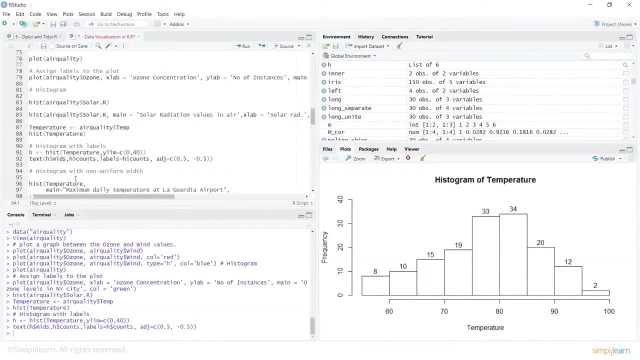 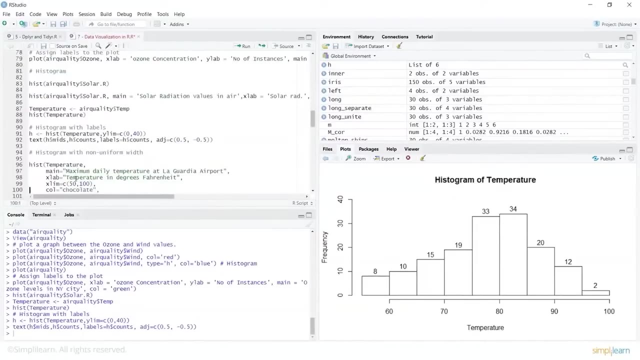 of values. it gives me the labels. now you can have a histogram with non uniform width, so you could do that by doing a hist function and then passing in your temperature. you can say what will be the main, what is the title, what will be your x lab. 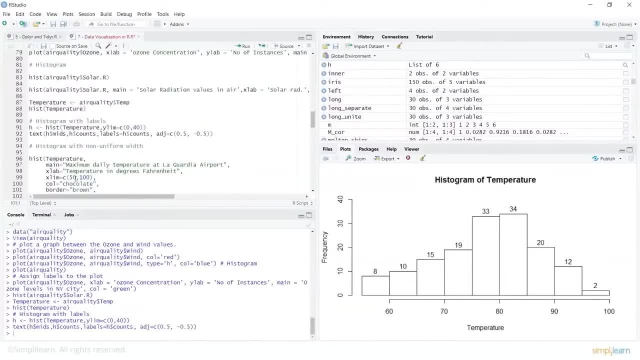 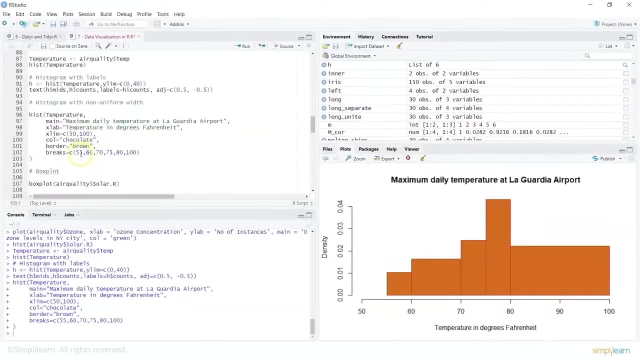 it will tell you a limit around x axis, what is the color, what is the border, what are the breaks you would want to have for your bars, and you can simply create a histogram using this. so this basically takes the breaks which we have given, such as 55 to 60. 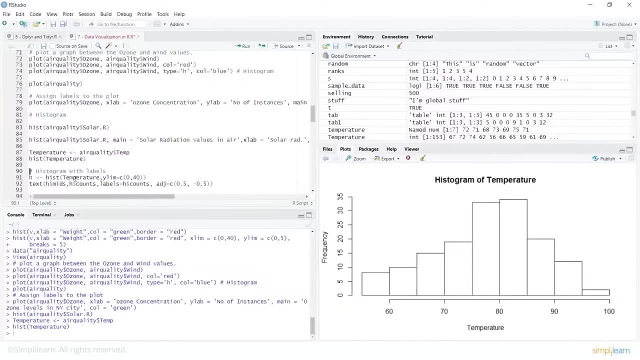 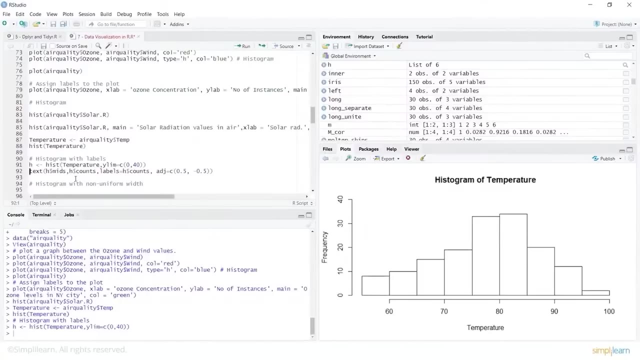 the frequency of the temperature values and what values have the most frequency or most difference. now you can create a histogram with labels, so let's do that with the limit, and then let's also use text to basically give in the values, which also takes the values and for 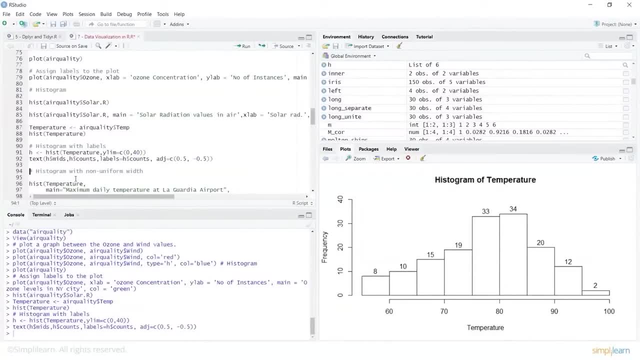 each set of frequency or each set of values. it gives me the labels. now you can have a histogram with non uniform width, so you could do that by doing a hist function and then passing in your temperature. you can say what will be the mean. what is the title? 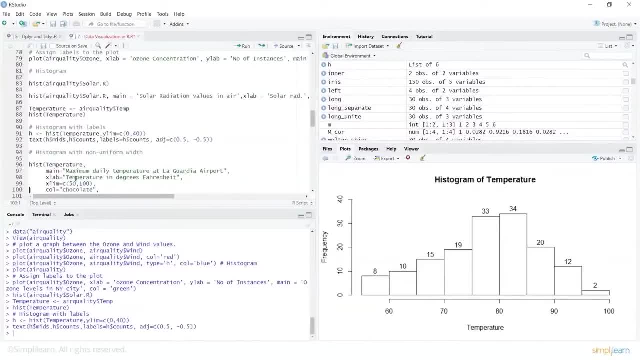 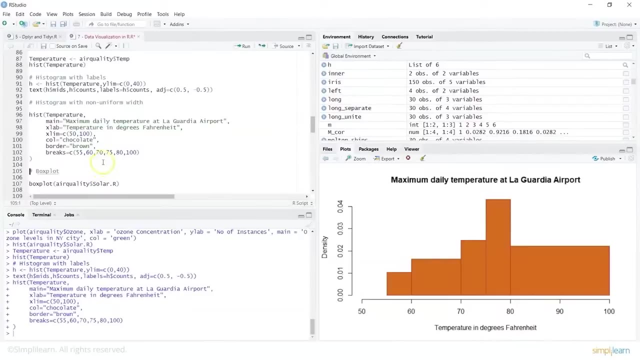 what will be your x lab. it will tell you a limit around x axis, what is the color, what is the border, what are the breaks you would want to have for your bars, and you can simply create a histogram using this. so this basically takes the breaks which we have given, such as: 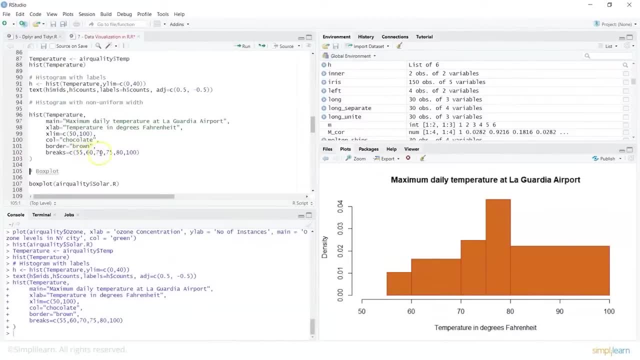 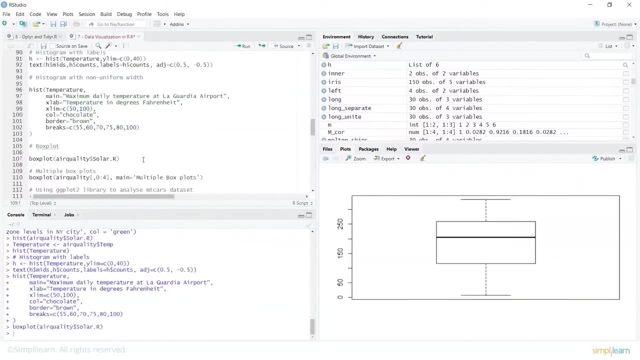 55 to 60, 60 to 70, 70 to 75 and so on. so this is basically creating a histogram with non uniform width, and it purely depends on the kind of values, what you have now. you can also create a box plot, which sometimes helps. 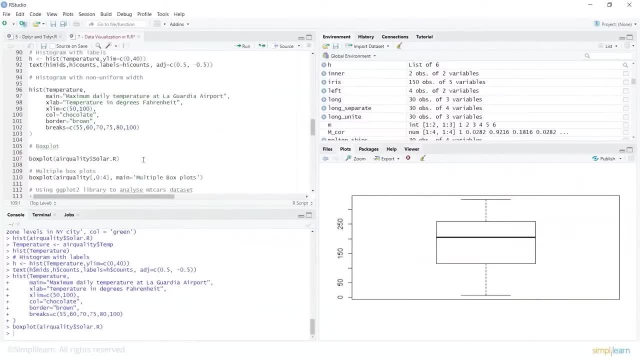 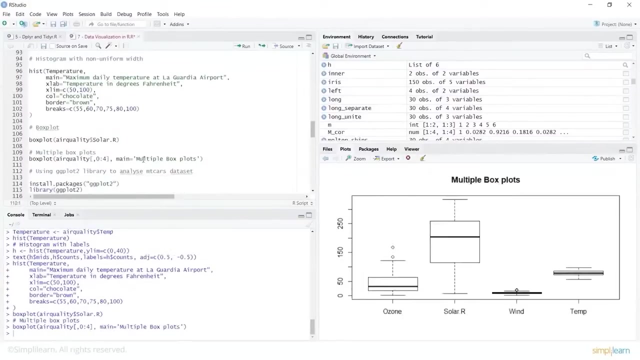 us in understanding the data quartiles, also understanding our outliers, so you can create multiple box plots based on the data from air quality. so we will select all the data and then we will do some slicing on the data. so let's create a box plot which tells: 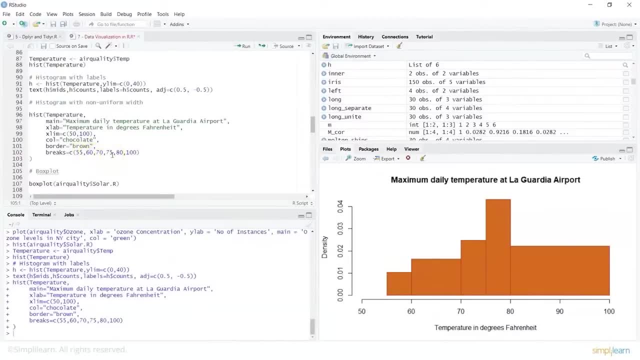 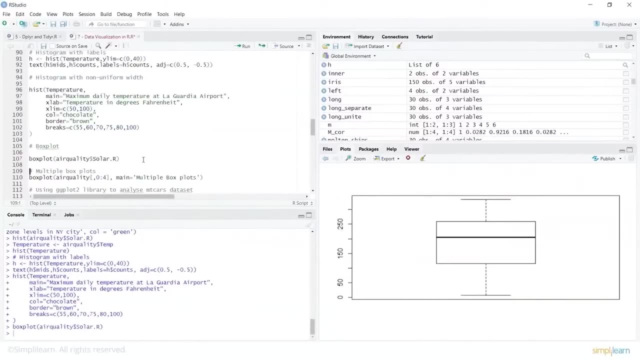 60 to 70, 70 to 75 and so on. so this is basically creating a histogram with non uniform width and it purely depends on the kind of values, what you have now. you can also create a box plot, which sometimes helps us in understanding the the data. 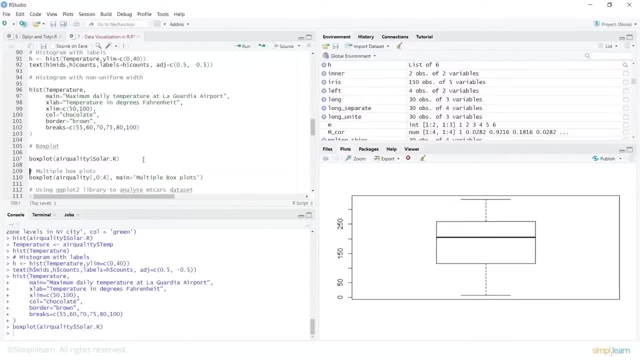 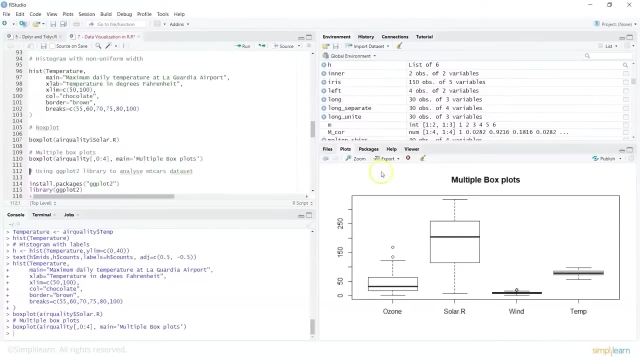 quartiles, also understanding our outliers. so you can create multiple box plots based on the data from air quality. so we'll select all the data and then we'll do some slicing on the data. so let's create a box plot which tells me the values and if you look at these, 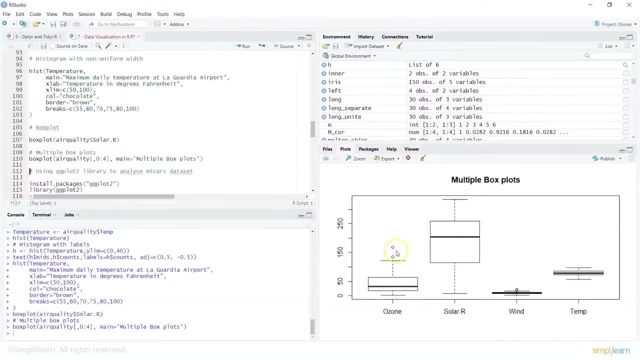 points here like single dots. these are basically your outliers. we can learn about that more in later sections. so you can use your ggplot2 library to analyze a particular data set. so for that we will first use the installpackages and get ggplot2. so it says: do you want to? 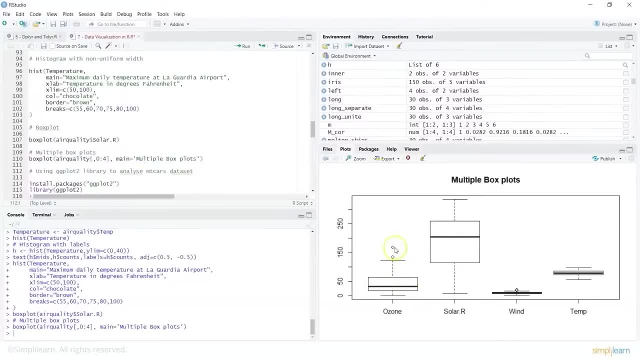 me the values, and if you look at these points here like single dots, these are basically your outliers. we can learn about that more in later sections, so you can use your ggplot2 library to analyze a particular data set. so for that we will first use the install. 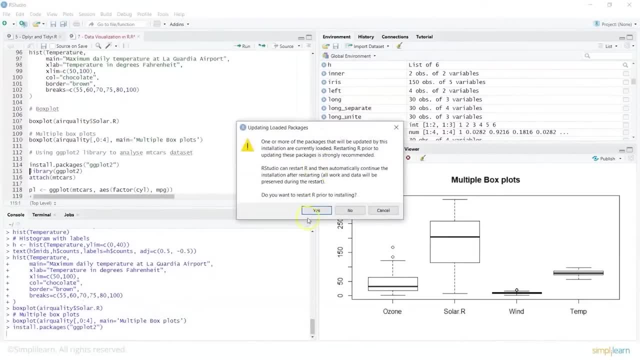 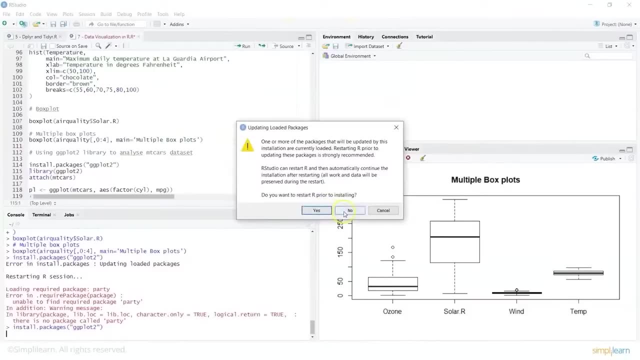 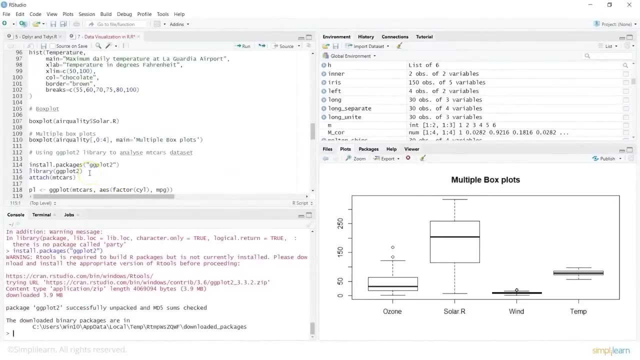 packages and get ggplot2. so it says: do you want to restart r? and i can say yes, so let it get the package. i think the package was already there, and now let's look at using ggplot2. so for that i have the library function. 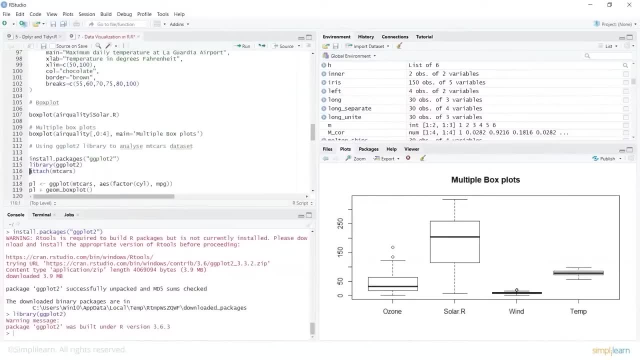 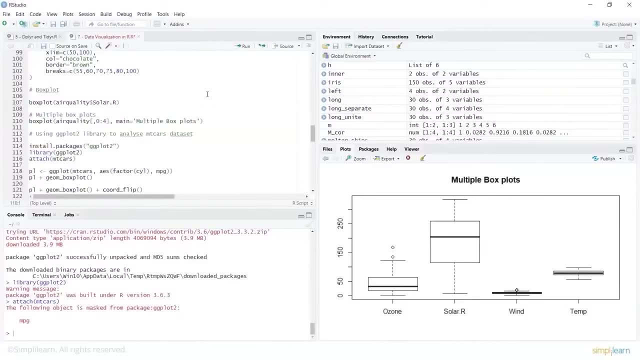 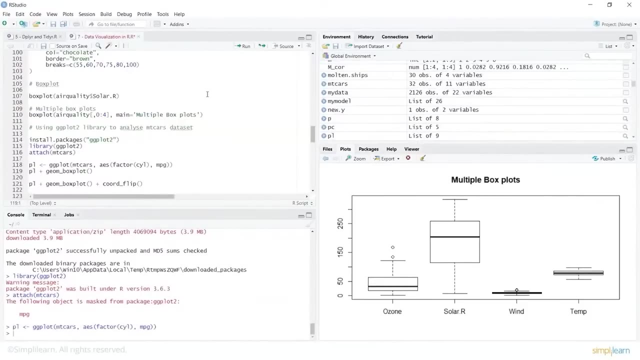 and let's do a attach where i am getting a data set which is empty cars. now then i will create a variable, p1, i will use ggplot, i will pass in my data, i will give the aesthetics, what is the columns which you would be interested in, and then 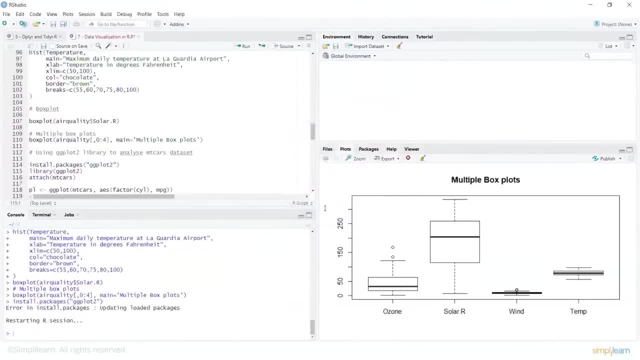 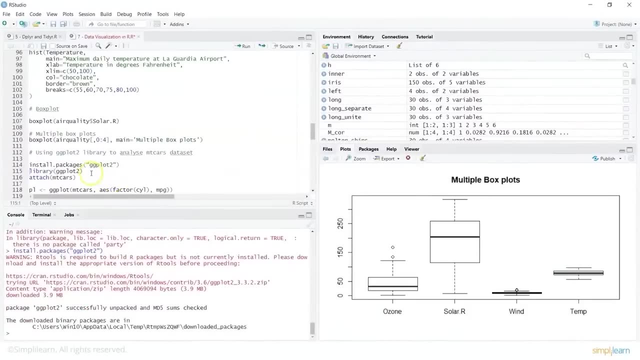 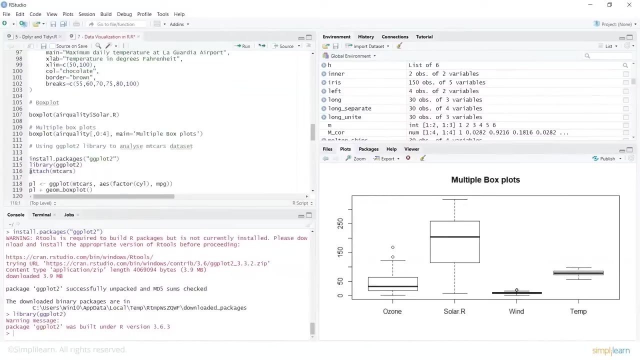 restart R and I can say yes, so let it get the package. I think the package was already there and now let's look at using ggplot2. so for that I have the library function and let's do a attach where I am getting a data set which is empty cars. 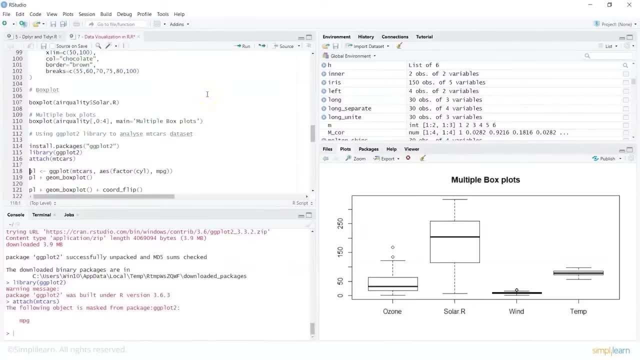 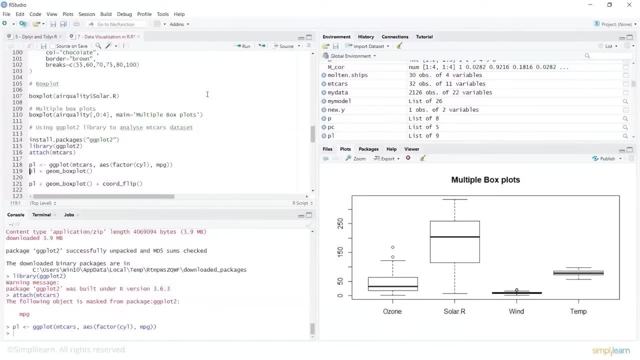 now. then I will create a variable p1, I will use ggplot2, I will pass in my data, I will give the aesthetics, what is the columns which you would be interested in, and then you are using geom underscore box plot to basically create a plot which gives me. 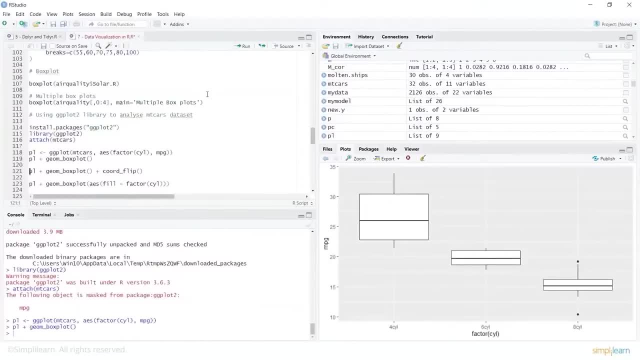 the box plot for the values here, and this is based on the cylinders which is there in your data, so we can always look at what does our data contain and what kind of values or features are available in the data. now let's create a box plot. we will also use the 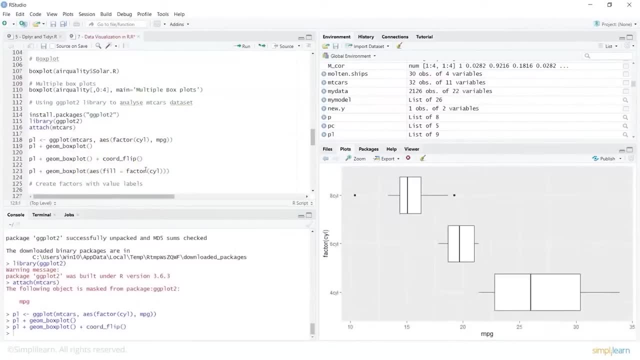 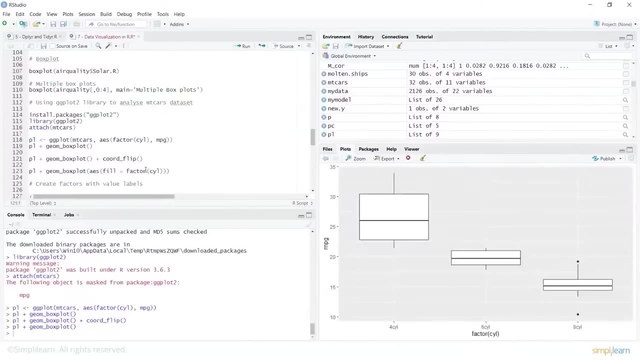 coordinate function and that basically gives me based on the data. so I have changed the coordinates. now, if you look at the previous one, where we created a plot, we had mileage on the y axis and cylinders on the x axis. now I did a coordinate flip and that's like your transpose function. 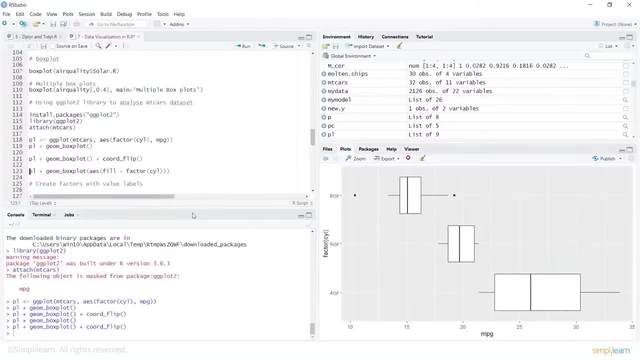 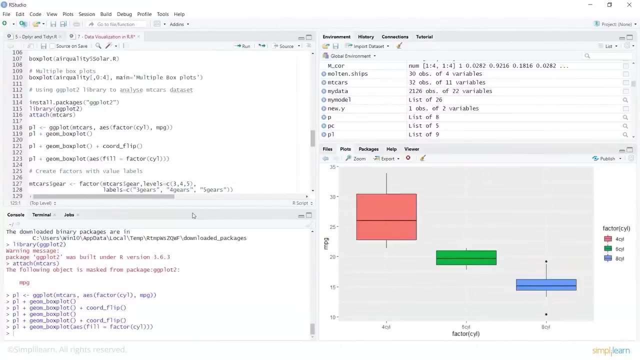 so you have created the box plot, but you have just flipped the coordinates. you can create a box plot and then say fill which is the factor of cylinder, so that can be used to fill up the values in your box plot. now what we can also do is: 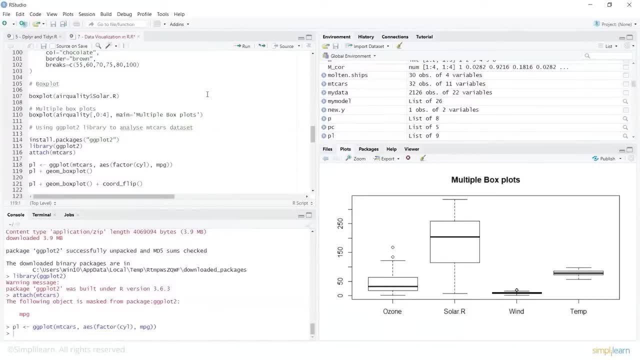 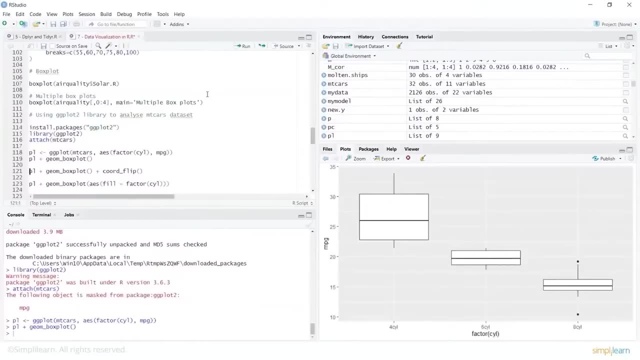 you are using geom underscore boxplot to basically create a plot which gives me the boxplot for the values here, and this is based on the cylinders which is there in your data, so we can always look at what does our data contain and what kind of values or features. 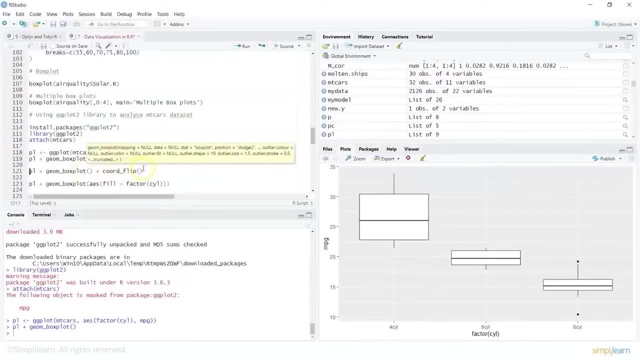 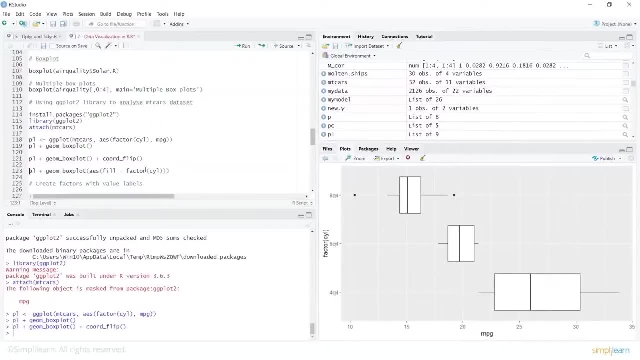 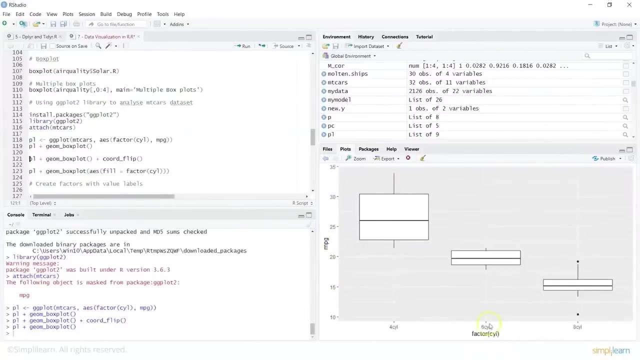 are available in the data. now let's create a boxplot. we will also use the coordinate function and that basically gives me based on the data. so i have changed the coordinates. now, if you look at the previous one, where we created a plot, we had mileage on the y-axis. 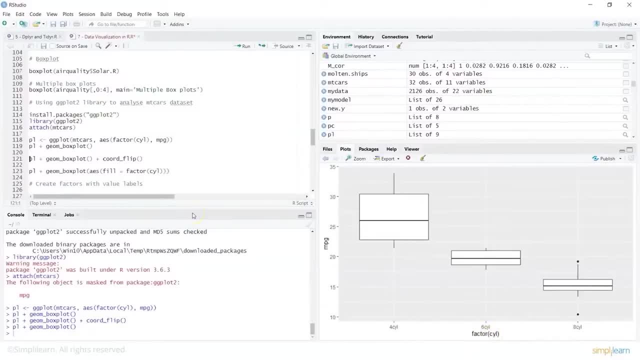 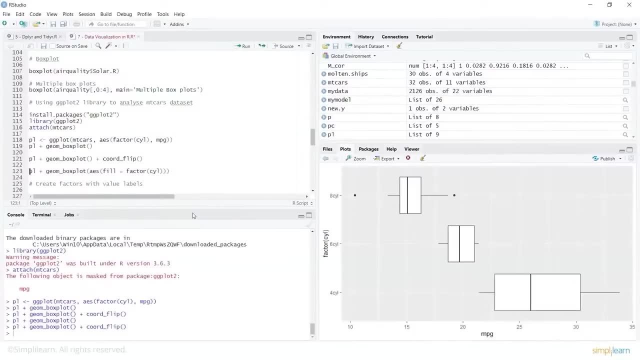 and cylinders on the x-axis. now i did a coordinate flip and that's like your transpose function. so you have created the boxplot, but you have just flipped the coordinates. you can create a boxplot and then say fill, which is the factor of cylinder, so that can be used to fill up the 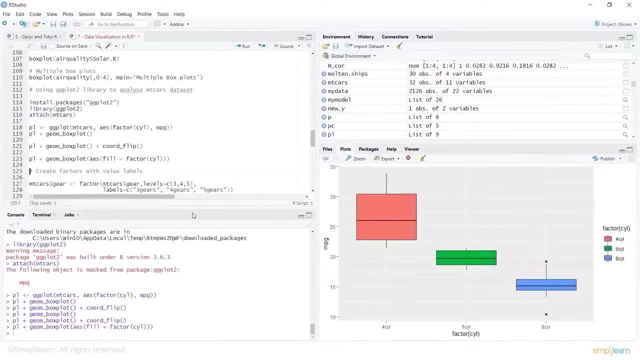 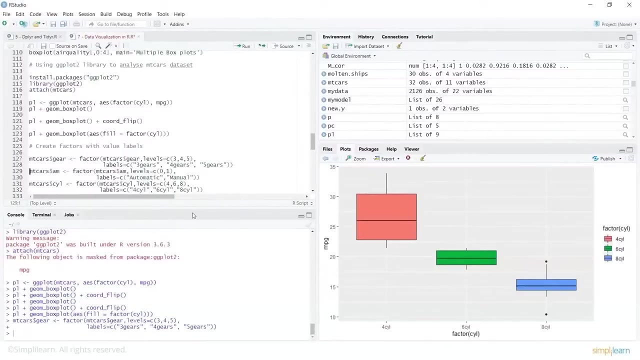 values in your boxplot. now, what we can also do is we can create factors. so we have learnt about factors earlier, which is usually used to work on categorical variables. so here let's create a factor which is empty: cars, gear you have am, you have cylinder, and if you look at 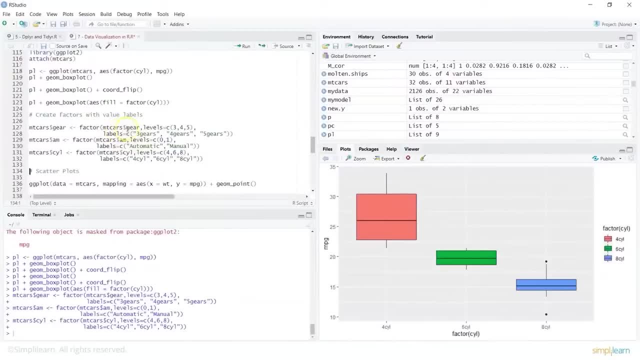 the factors which we have created. we have passed our data. what is the field or the column we are interested in, what is the level of values there and what are the labels for those values? so we have learnt about factors. you can always look into the previous section and learn more. 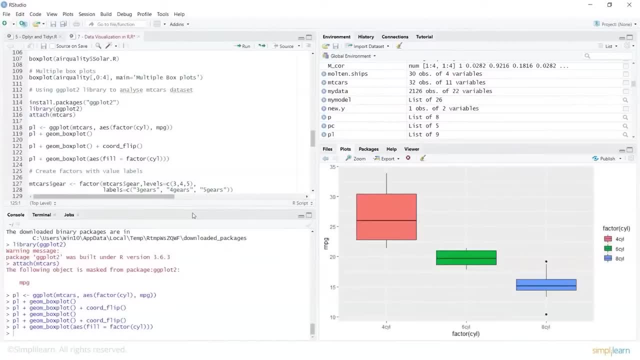 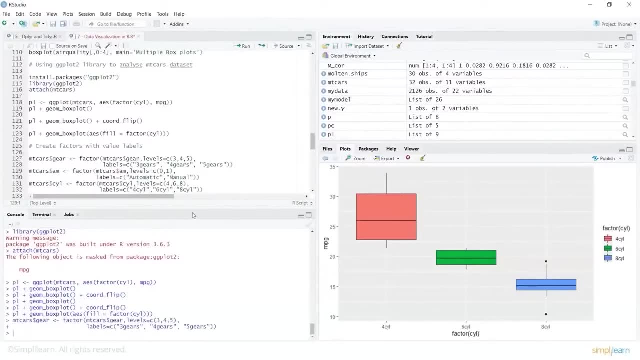 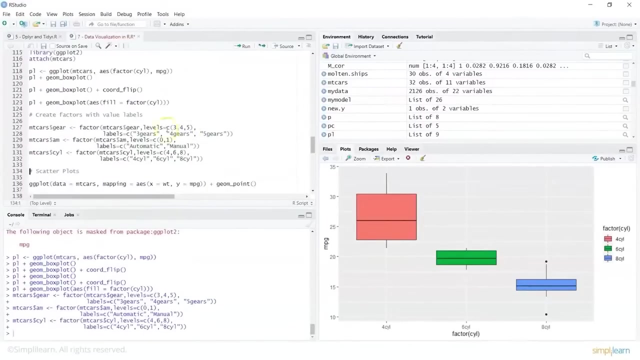 we can create factors. so we have learnt about factors layer, which is usually used to work on categorical variables. so here let's create a factor which is empty cars, gear you have am, you have cylinder, and if you look at the factors which we have created, we have: 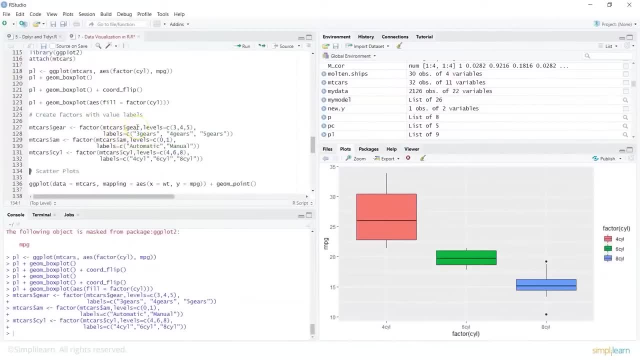 passed our data. what is the field or the column we are interested in? what is the level of values there and what are the labels for those values? right, so we have learnt about factors. you can always look into the previous section and learn more about factors. now let's create. 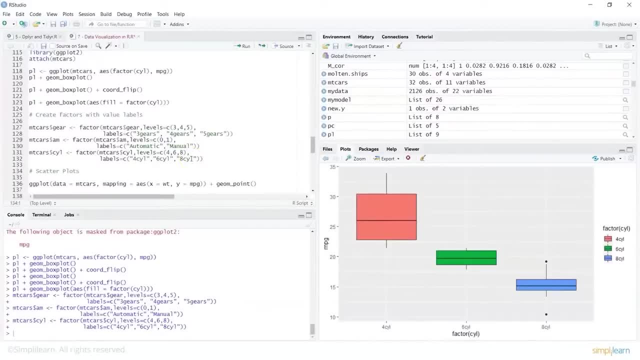 about factors. now let's create a scatterplot by using the ggplot function. again, we will use the data as empty cars. i will go for mapping option and then i will give my aesthetics. that is what would be x, what would be your y and you also would want to use. 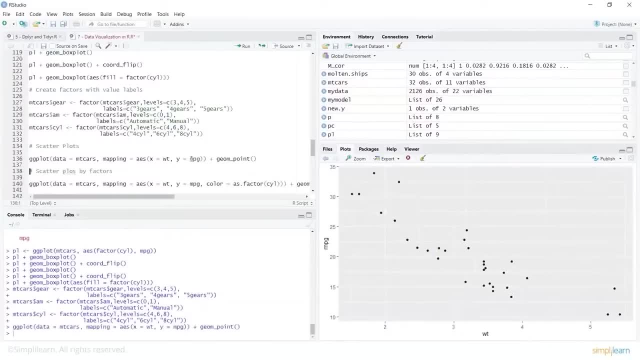 what kind of function you are using. so let's go for geom point, and that basically helps me in creating a scatterplot. now you can create a scatterplot by factors, so here we will say ggplot. so notice, in all of these cases, depending on the kind of data you have, 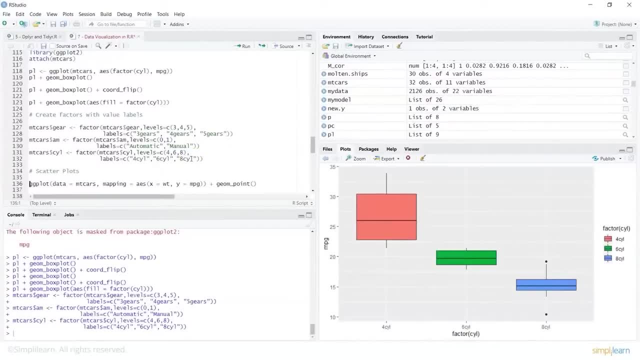 a scatter plot by using the ggplot function. again, we will use the data as empty cars. I will go for mapping option and then I will give my aesthetics. that is, what would be x, what would be your y and you also would want to use what kind of function you are. 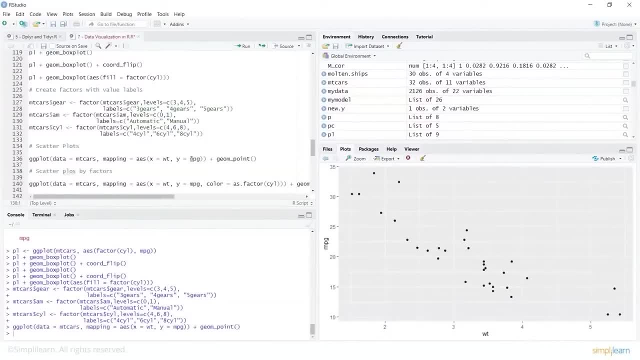 using. so let's go for geom point and that basically helps me in creating a scatter plot. now you can create a scatter plot by factors, so here we will say ggplot. so notice, in all of these cases, depending on the kind of data you have, depending on the kind of plot you are interested, 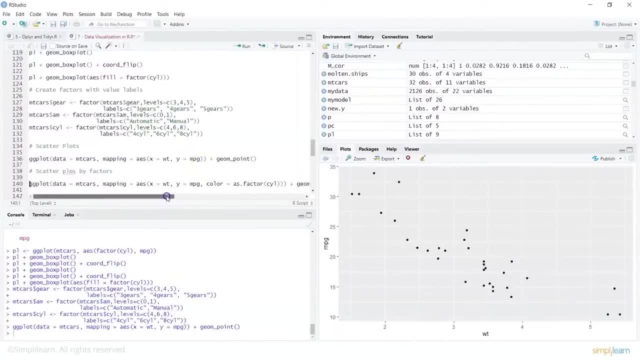 in. you will use the ggplot and then basically a function with that or the inbuilt package. so here I am saying: data is empty cars. I am going for mapping which basically will take the values for your x and y, what is the color and the coloring will. 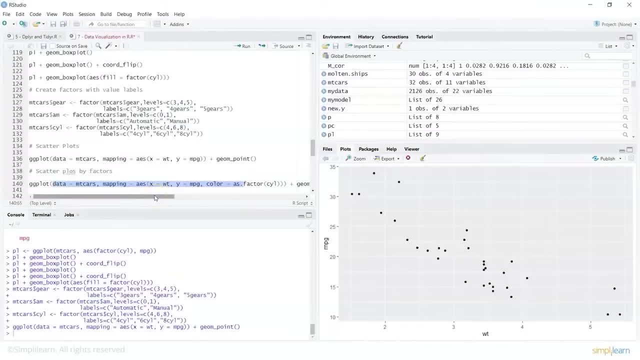 be done based on the factor values. now, if you remember, factors will obviously have some levels and those levels will basically help you in differentiating between your categorical variables. so I am saying as dot factor on cylinder, and then I am using geom point to basically create the scatter plot. so let's. 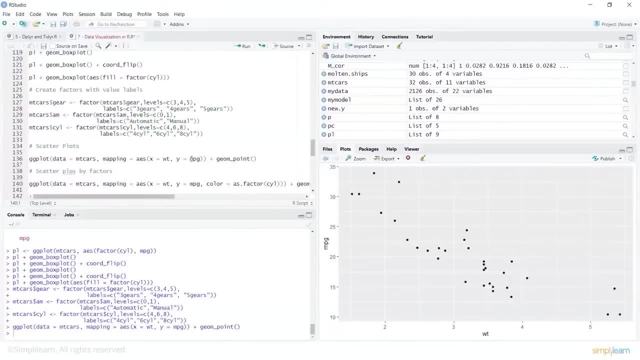 depending on the kind of plot you are interested in, you will use the ggplot and then basically a function with that or the inbuilt package. so here i am saying data is empty cars. i am going for mapping which basically will take the values for your x and y. what? 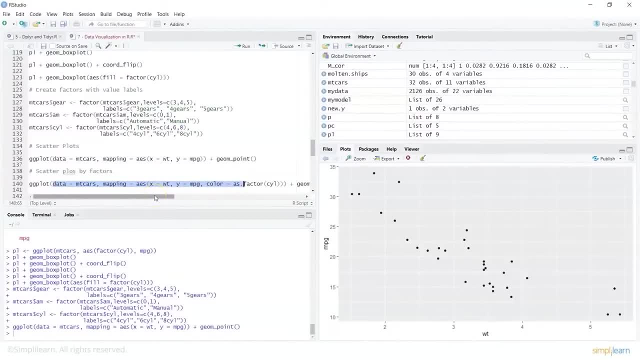 is the colour, and the colouring will be done based on the factor values. now, if you remember, factors will obviously have some levels and those levels will basically help you in differentiating between your categorical variables. so i am saying as dot factor on cylinder and then i am using geom point. 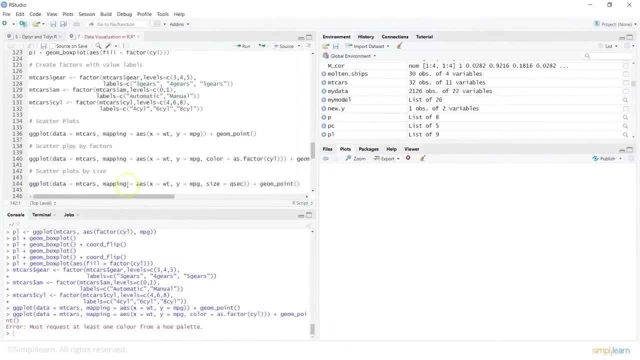 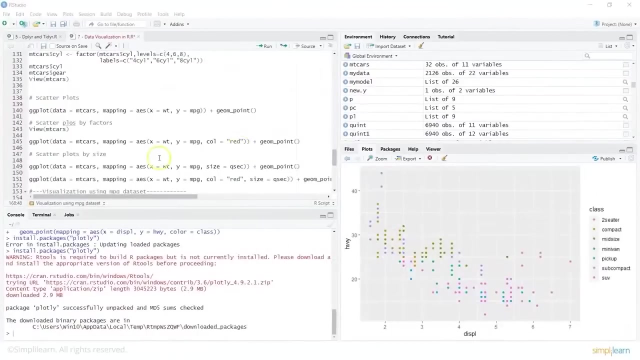 to basically create the scatterplot. so let's do this. and i can look at the values of this one. so it says: must be. there is an error which says must at least one colour from the hue palette. so let's look at that one. so the error which 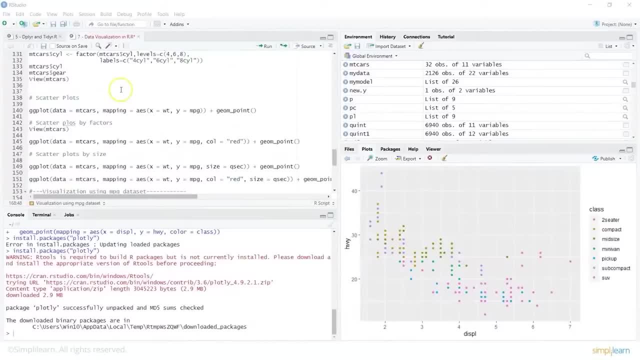 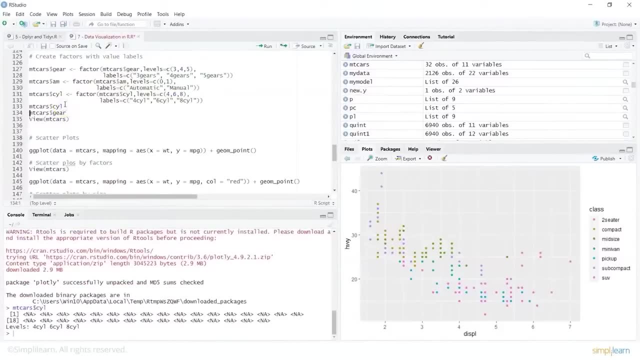 we were facing when we gave colour as the factor values was because when you look at these factors which were created with some labels, if we look at the values of these, it tells me there are any values in that particular column, similarly your gear, or similarly you can completely look at the 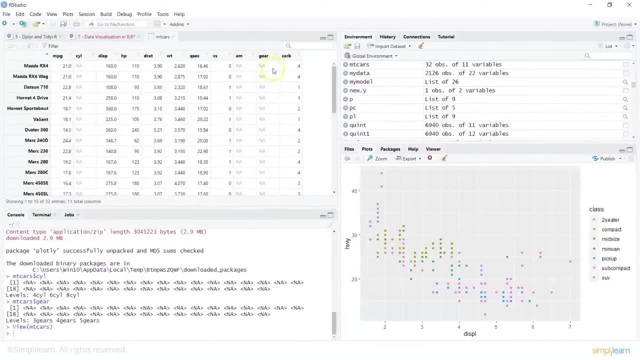 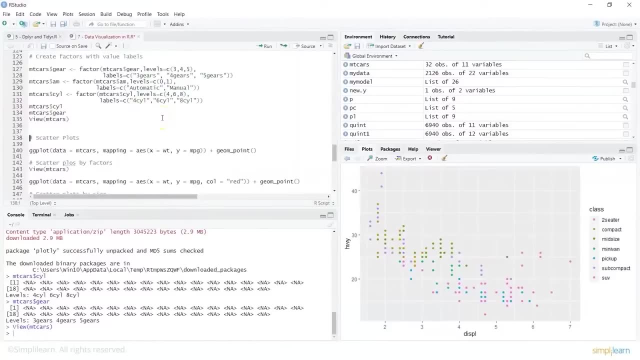 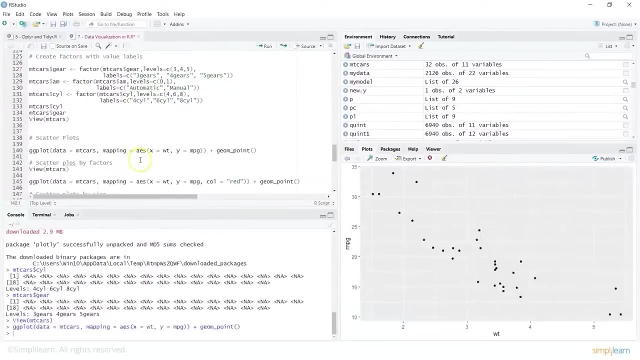 complete data set. it tells me: cylinder you have, am you have gear. now these have some. we have created some labels, but these have any values. so what we can do is we can create a scatterplot, as we did earlier, by giving the aesthetics, and that's a simple scatterplot. 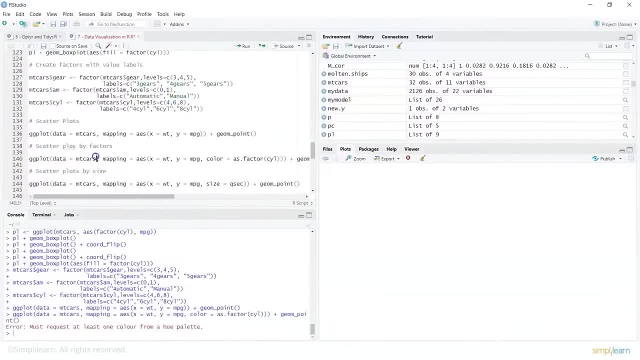 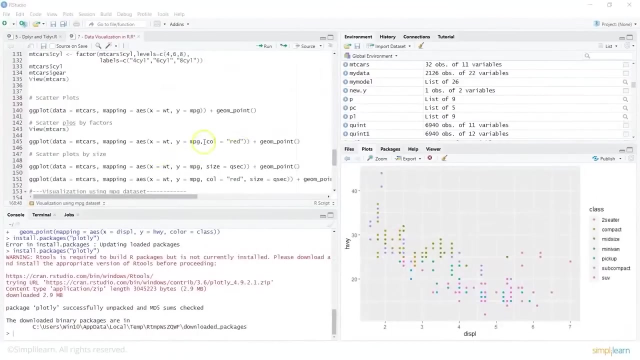 do this and I can look at the values of this one. so it says: must be. there is an error which says must at least one color from the hue palette. so let's look at that one. so the error which we were facing when we gave color as the factor values was: 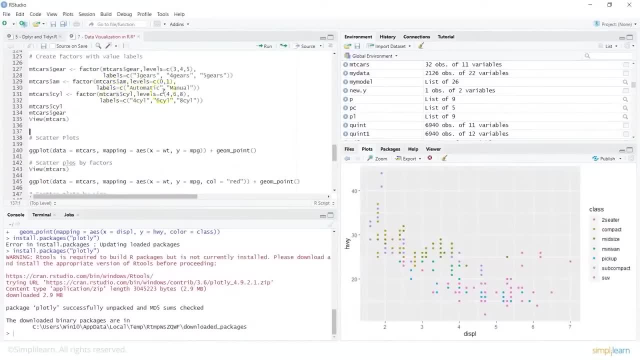 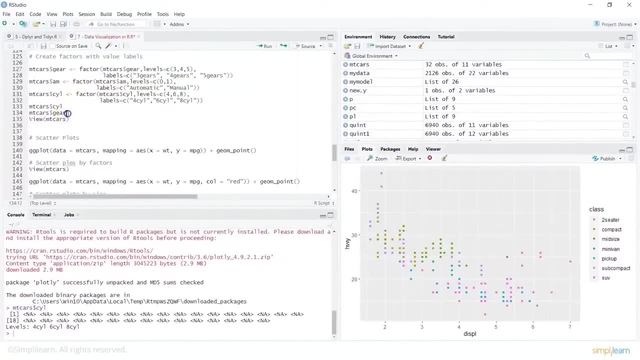 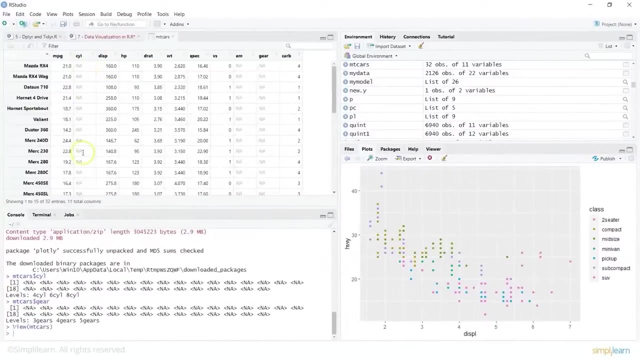 because when you look at these factors which were created with some labels, if we look at the values of these, it tells me there are any values in that particular column, similarly your gear. or similarly you can completely look at the complete data set. it tells me: cylinder you have, am you have gear? 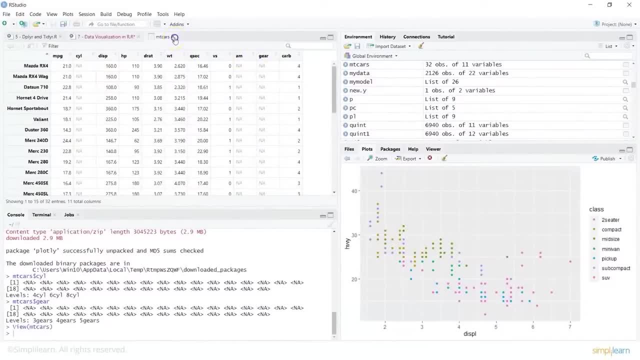 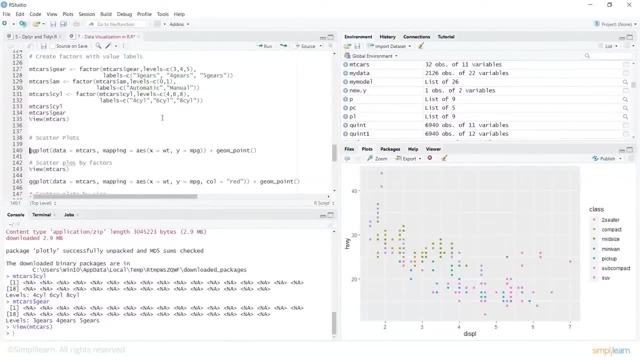 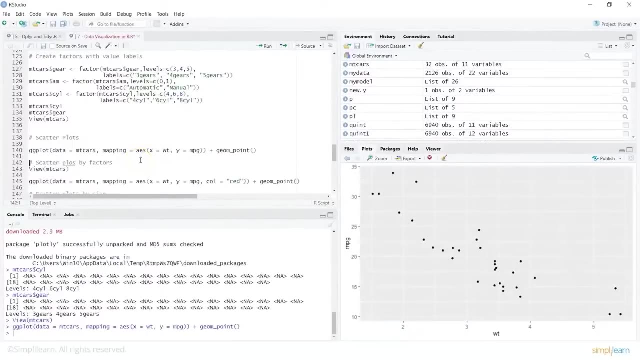 now, these have some. we have created some labels, but these have any values. so what we can do is we can create a scatter plot, as we did earlier, by giving the aesthetics, and that's a simple scatter plot wherein I am also using geom point so that I can have 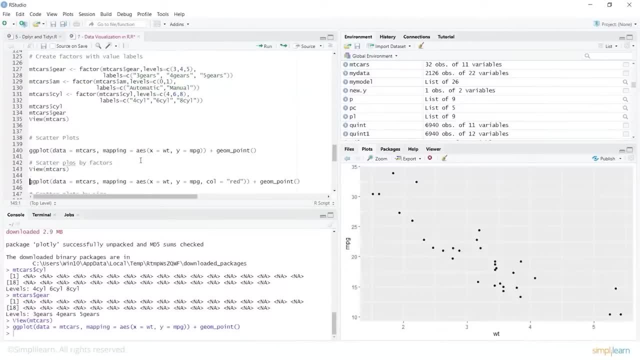 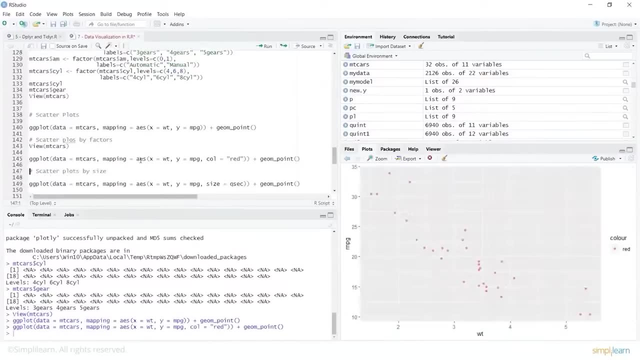 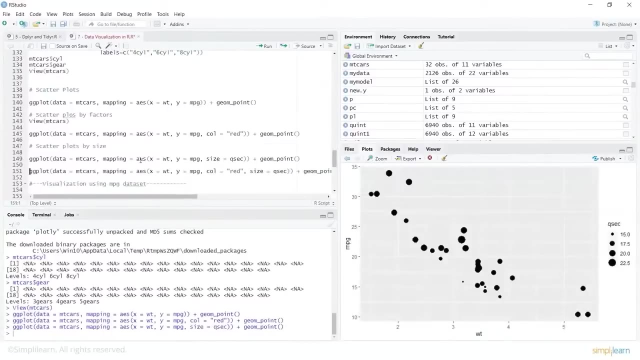 these points by defaults or with defaults. you can also give a color specific. basically, if you would want to have different kind of data in the same plot, or I can create scatter plots by different sizes by giving a size, or I can give a color and size and 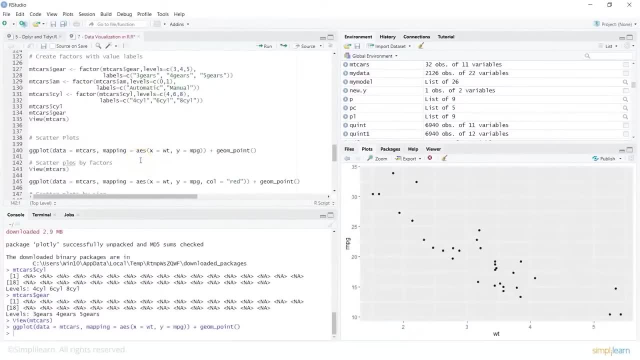 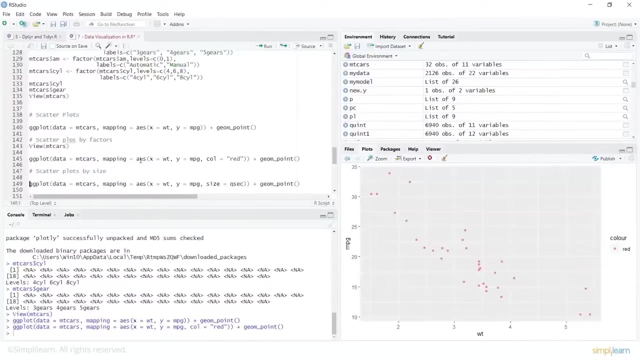 wherein i am also using geom point, so that i can have these points by defaults or with defaults. you can also give a colour specific, basically, if you would want to have different kind of data in the same plot, or i can create scatterplots by different sizes by 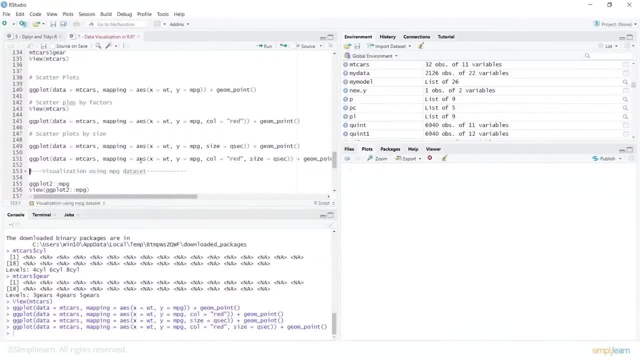 giving a size, or i can give a colour and size, and that's again one way in which you can create your scatterplots. now let's also see how you can visualize one more data set, which is gg. so i can also do it in this way, where i 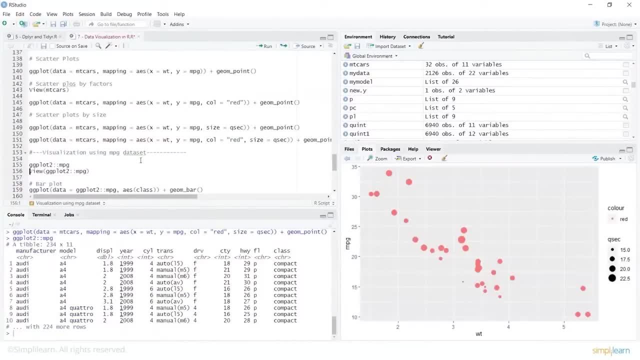 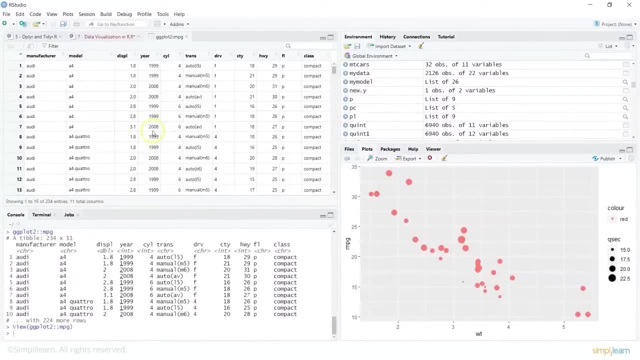 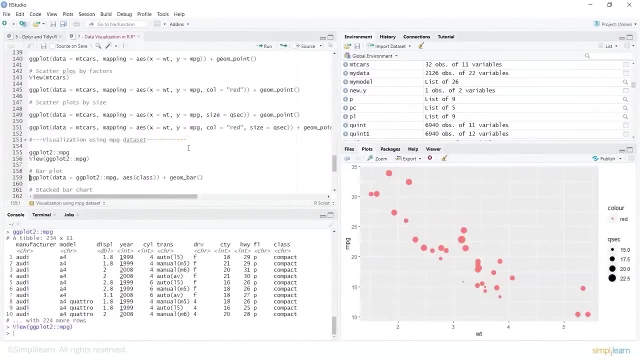 set gg, plot 2, and then pass and look at the data set. what we have here. you can just do a view on this to see what my data contains, if the fields have any any values, if that's going to affect your plotting. so now what we can do is we can create a bar plot. 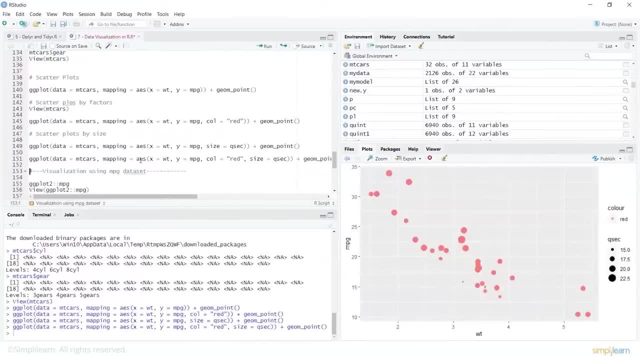 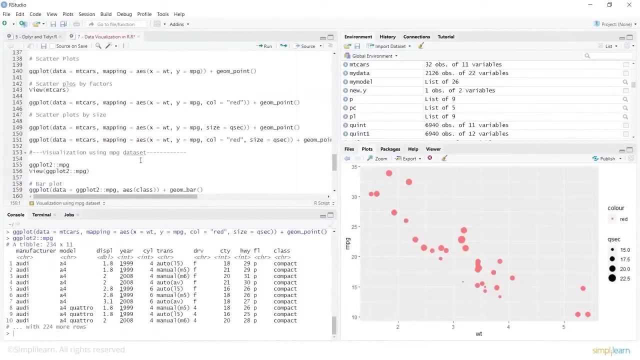 that's again one way in which you can create your scatter plots. now let's also see how you can visualize one more data set, which is mpg. so I can also do it in this way, where I said ggplot2 and then pass in. look at the data set. what? 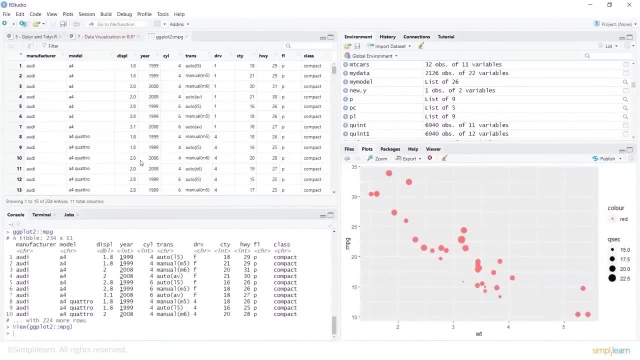 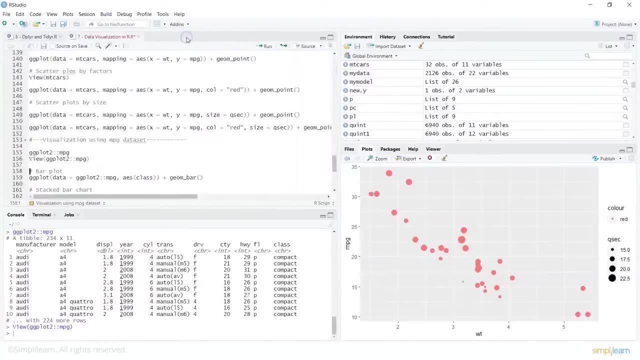 we have here. you can just do a view on this to see what my data contains, if the fields have any values, if that's going to affect your plotting. so now what we can do is we can create a bar plot or a bar chart. so I am saying 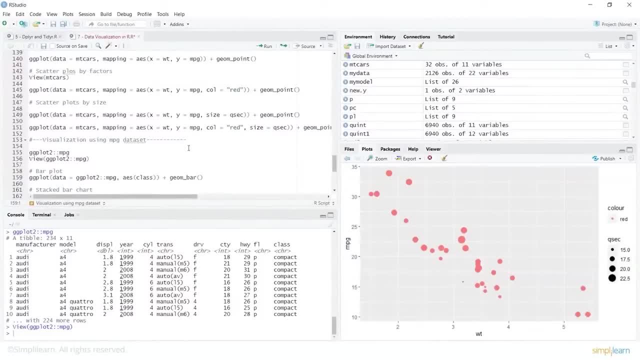 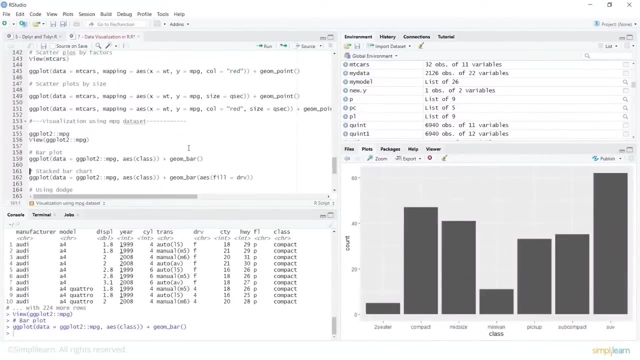 ggplot, the data would be as we have given in previous lines, that is, ggplot2 mpg. then I will say what should be in my aesthetics and what kind of chart are you going to create. so I am saying geom underscore bar. so that's my bar chart. 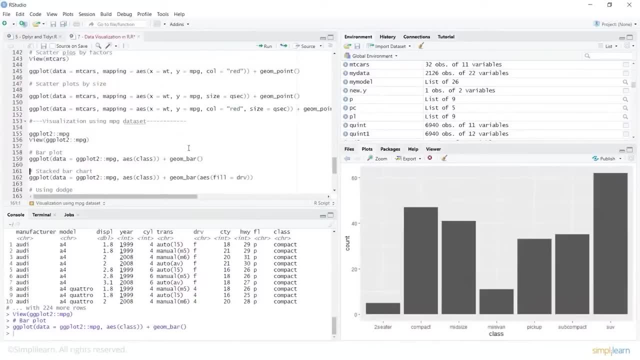 and that has basically your class and count. now you can create a stacked bar chart where your information is stacked in the same bars and we are still using the same data. we are going for aesthetics, which is class, and then when you say geom bar, which creates your stacked bar, we will use. 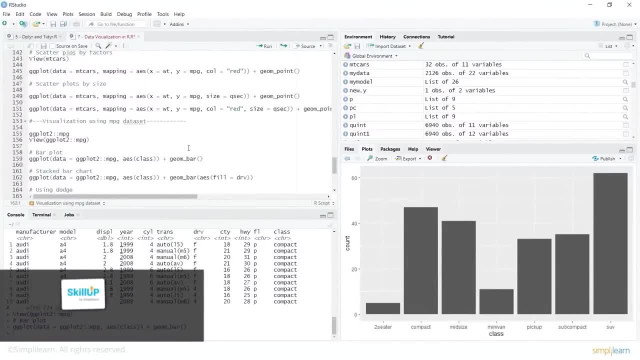 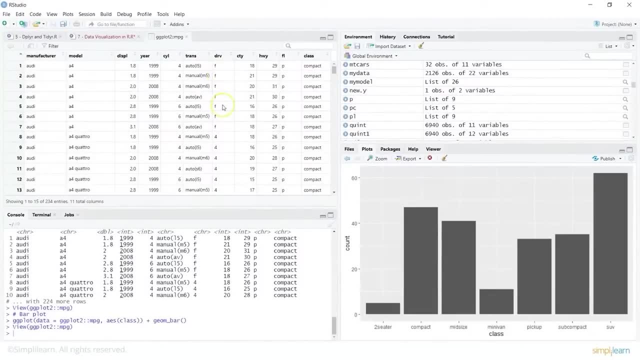 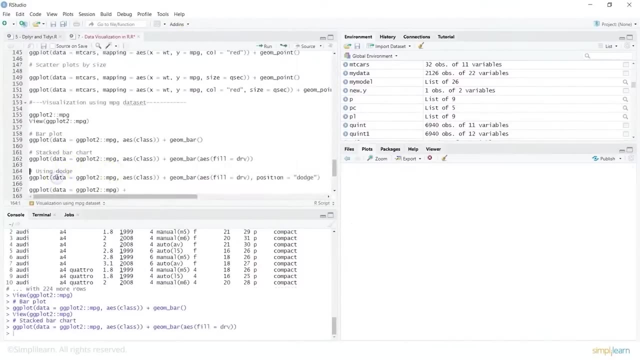 fill, which is drive, and we can always go back and look at our data, for example, you can always look into this. so you have the drive column here and you are also working on this complete data set, so let's go ahead and create a stacked bar chart. 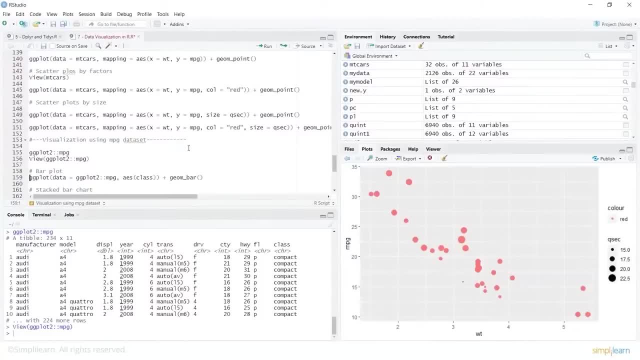 or a bar chart. so i am saying gg plot. the data would be as we have given in previous lines, that is, gg plot, 2 mpg. then i will say what should be in my aesthetics and what kind of chart are you going to create. so i am saying gom underscore. 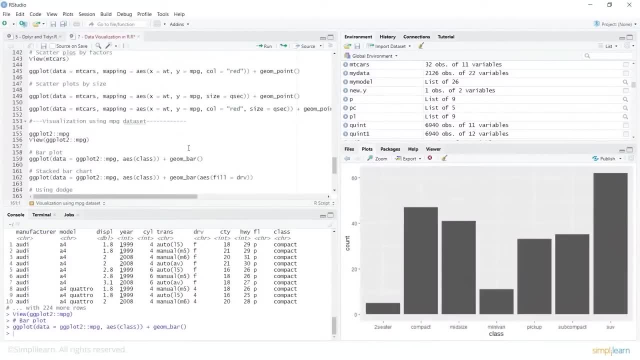 bar. so that's my bar chart and that has basically your class and count. now you can create a stacked bar chart where your information is stacked in the same bars and we are still using the same data. we are going for aesthetics, which is class, and then when you say gom bar, which 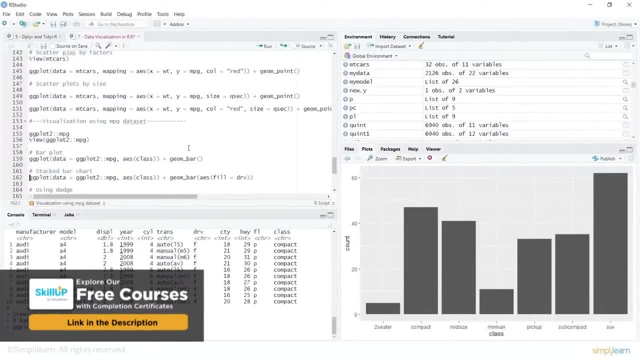 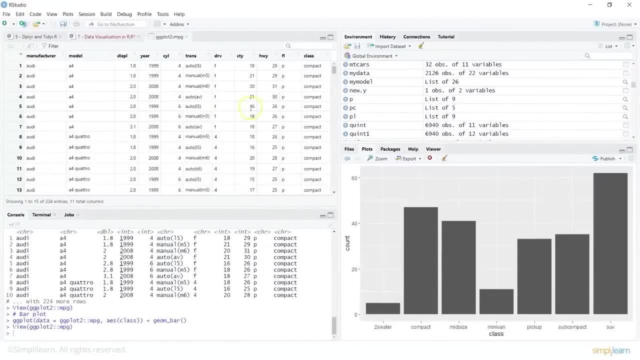 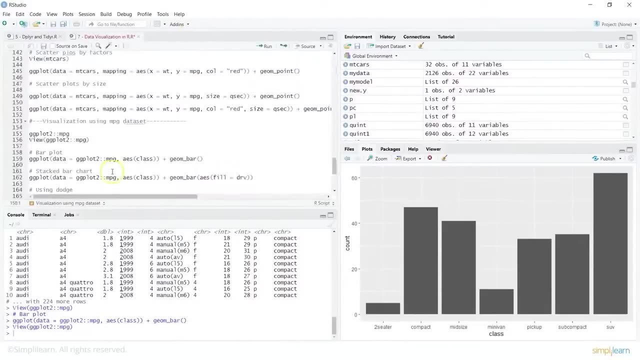 creates your stacked bar. we will use fill, which is drive, and we can always go back and look at our data. for example, you can always look into this. so you have the drive column here and you are also working on this complete data set. so let's go ahead and create a stacked bar. 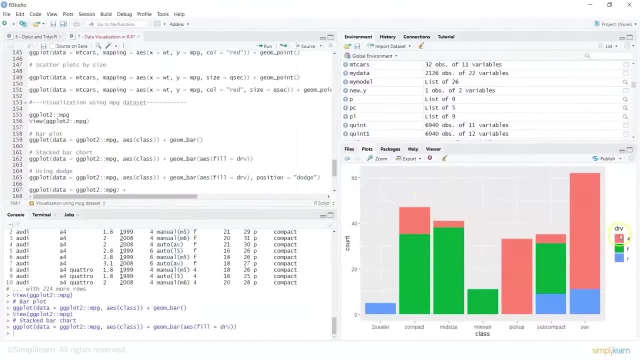 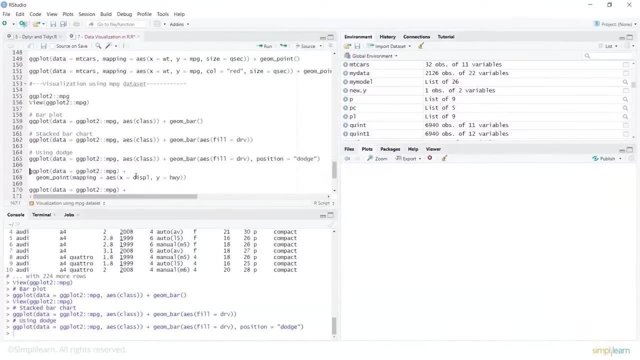 chart and that basically gives me the information where you have the drive information which is stacked here. now you can do a dodge by giving the position as dodge. so we are still going to go for a stacked chart, but this time the bars will be next to each other. 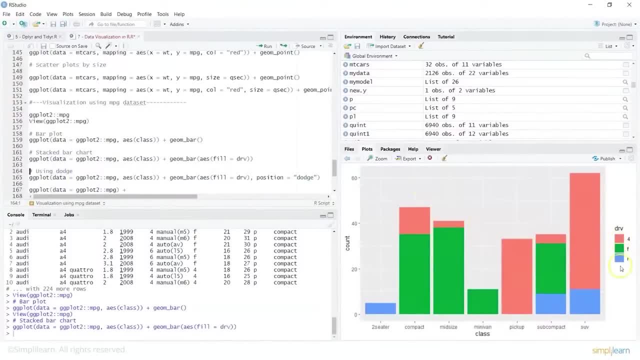 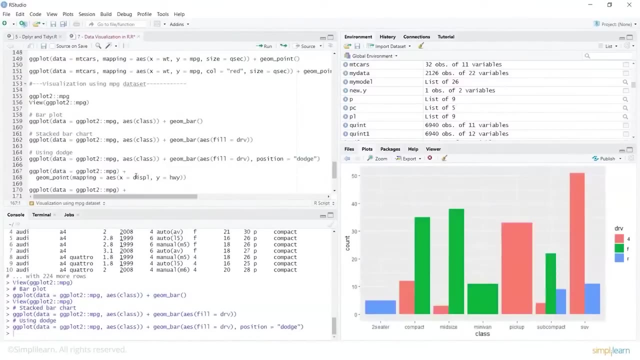 and that basically gives me the information where you have the drive information which is stacked here. now you can do a dodge by giving the position as dodge. so we are still going to go for a stacked chart, but this time the bars will be next to each other, and that. 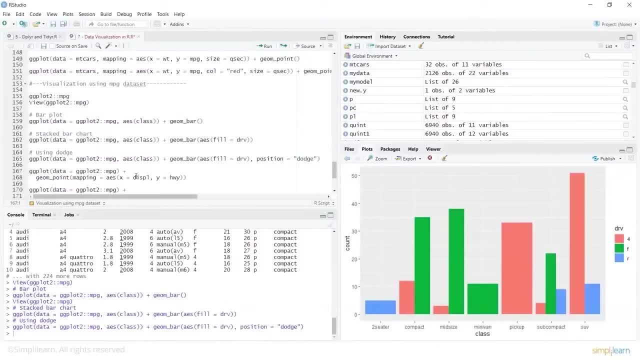 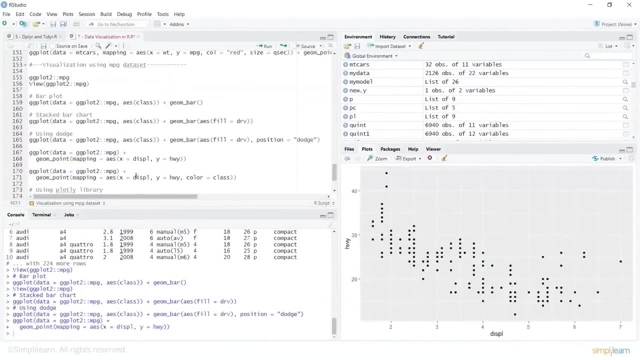 can also be done, which is very useful. you can use this by using geom point, where you are mapping and you are specifying what are your aesthetics. so we were creating a scatter plot. now you can also use or give more details where you can say color can be based on the class. 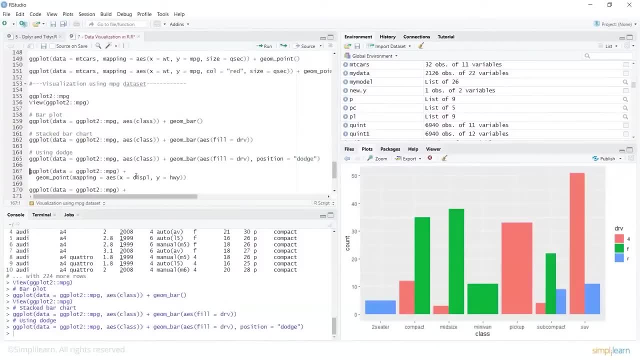 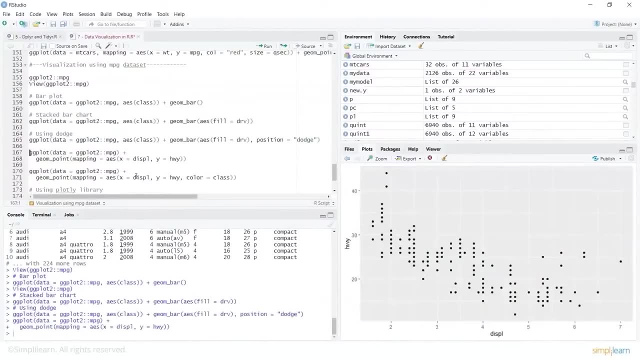 and that can also be done, which is very useful. you can use this by using gom point, where you are mapping and you are specifying what are your aesthetics. so we were creating a scatter plot. now you can also use or give more details where you can say color can be based on the 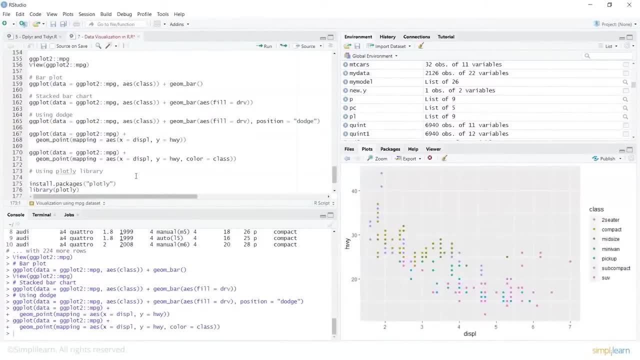 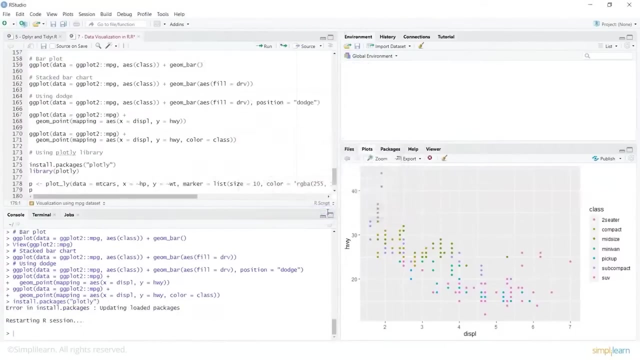 class and we have different classes and based on that, my points have been colored. now you can also use a plot ly or plotly library, so let's install this one. i will say yes. for example, let it basically restart so that all my packages are updated, then i can access that. 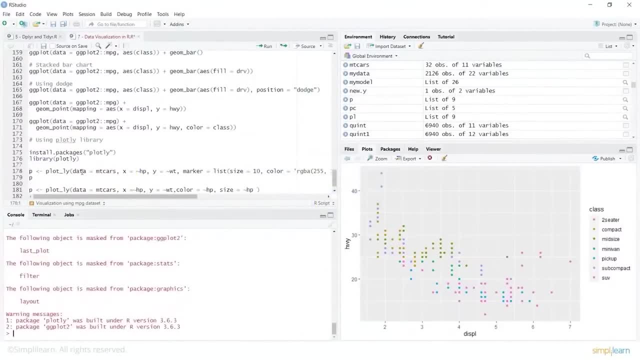 package, using library function, and then create a variable to which you are assigning your plot, underscore: ly plot, so data is empty. car, what will be your x axis, what will be your y axis and details on your marker which we have given, wherein i will give a list, which is size. 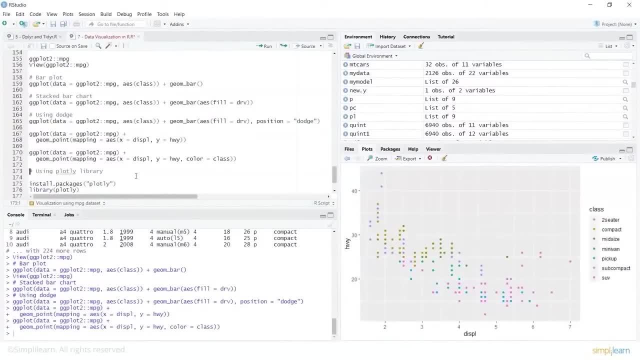 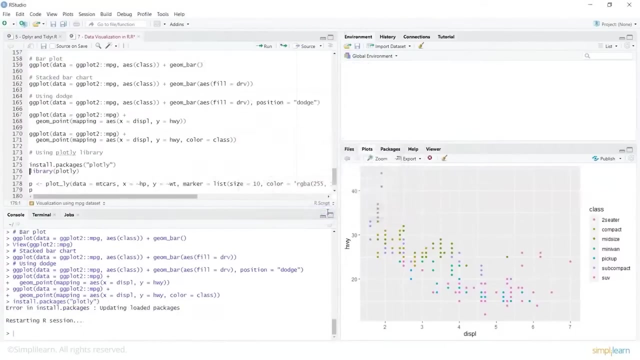 and we have different classes, and based on that, my points have been colored. now you can also use a plot ly or plotly library, so let's install this one. I will say yes, for example, let it basically restart so that all my packages are updated, then I can access that package. 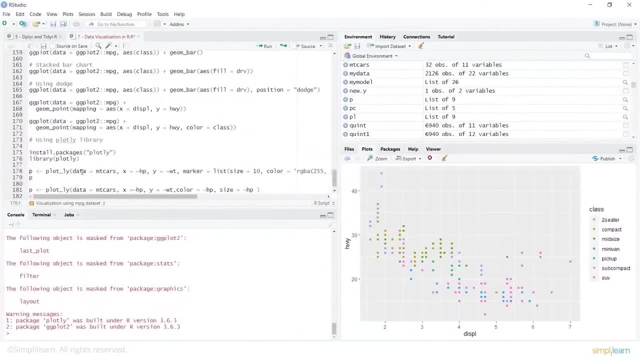 using library function and then create a variable to which you are assigning your plot, underscore: ly plot, so data is empty. cars, what will be your x axis, what will be your y axis and details on your marker which we have given, wherein I will give a list, which is size. 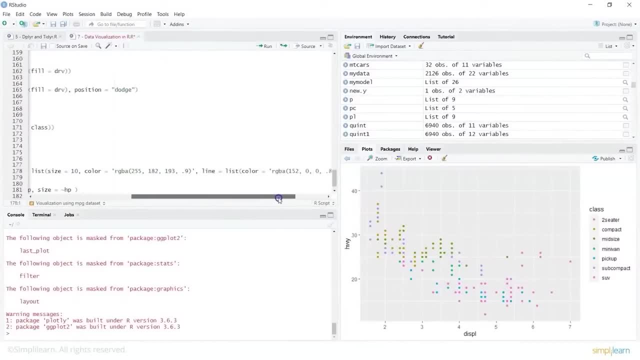 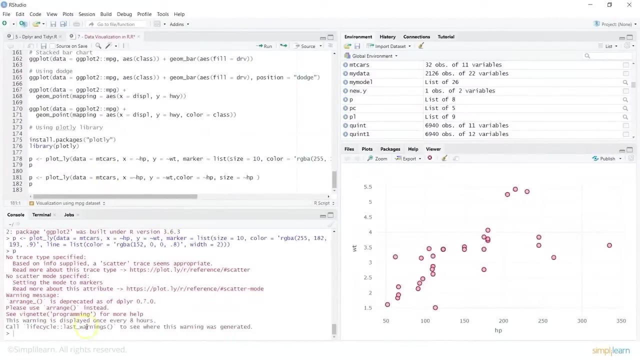 color, which is a combination, and then you have your line, what kind of color it will have and what will be the width. so this is where I am going to use plot ly, and let's look at this plot. so it basically gives me some information. now we 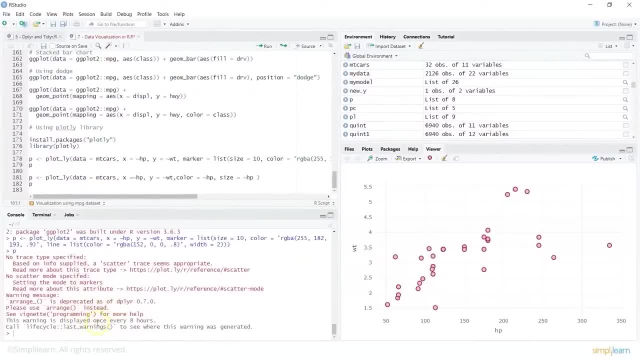 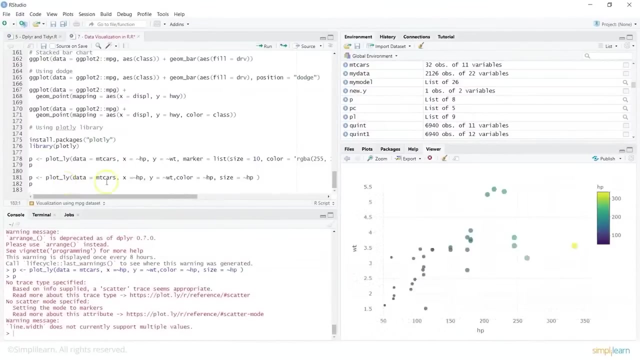 see some warnings which are getting generated, but there is, you don't need to worry about that. so you can look at the packages, what you have and what options you are using. so, similarly, we can create one more plot using plot ly and look at the values of those. 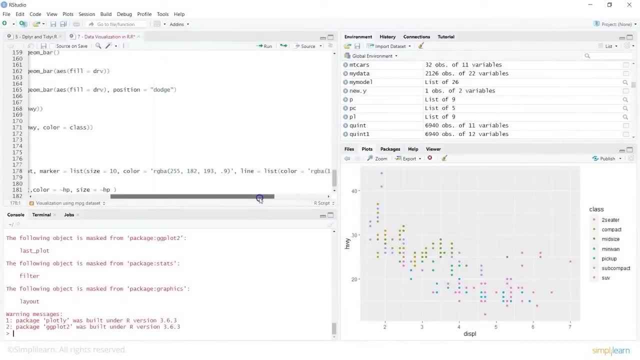 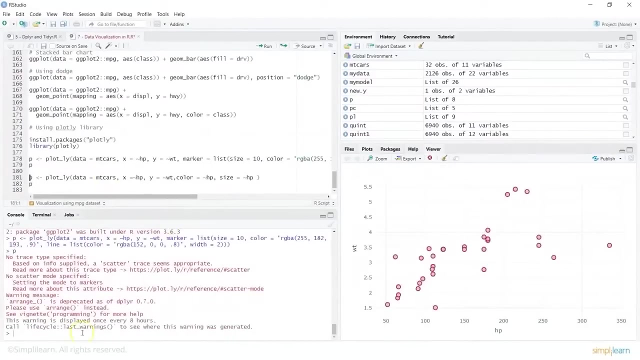 color, which is a combination, and then you have your line: what kind of color it will have and what will be the width. so this is where i am going to use plot ly and let's look at this plot. so it basically gives me some information. now we see some warnings which are going. 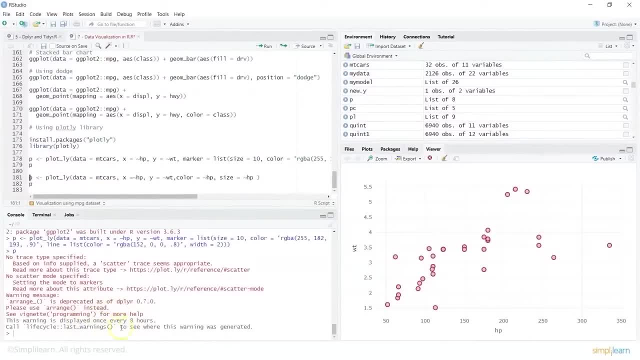 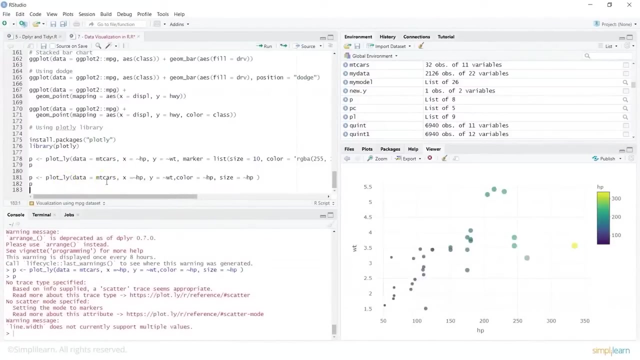 to be getting generated, but there is, you don't need to worry about that. so you can look at the packages, what you have and what options you are using. so, similarly, we can create one more plot using plot ly and look at the values of those. so that's a plot with a. 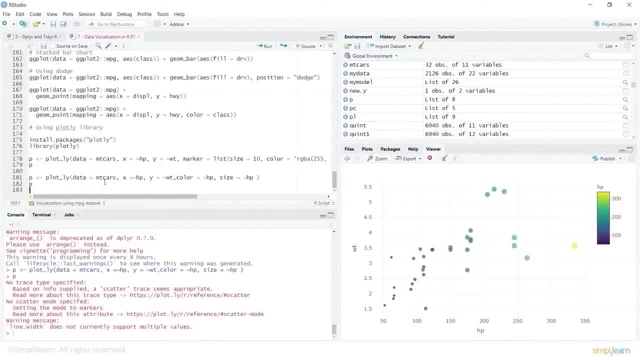 trend which explains me about my data. so this is a simple small tutorial on understanding, or how you can have your graphics or visualization used to understand your data. obviously, there are much more examples, much more ways in which you can pass into your plot functions or your gg plot. 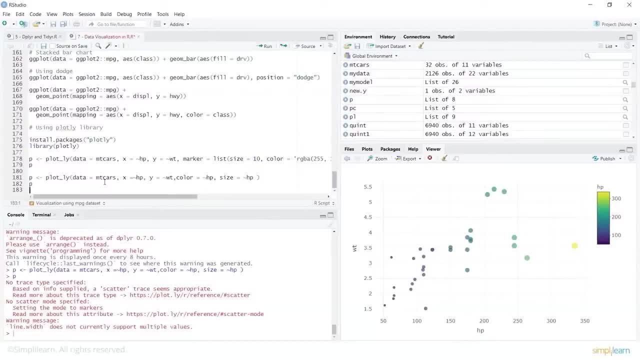 and the inbuilt packages which are available in R for your visualization. now that could be for exploratory data analysis or explanatory data analysis. so try these graphs and see if you can change these options and try or create new visualizations. good morning and good evening everyone so. 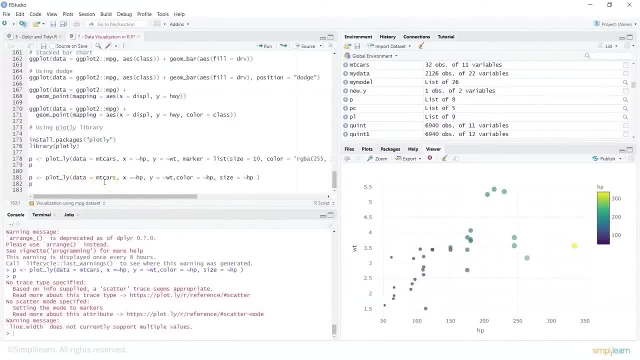 so that's a plot with a trend which explains me about my data. so this is a simple small tutorial on understanding, or how you can have your graphics or visualization used to understand your data. obviously, there are much more examples, much more ways in which you can pass into your 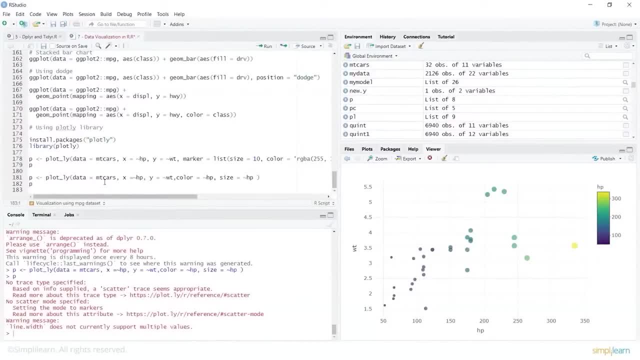 plot functions or your gg plot and the inbuilt packages which are available in R for your visualization. now that could be for exploratory data analysis or explanatory data analysis. so try these graphs and see if you can change these options and try or create new visualizations. 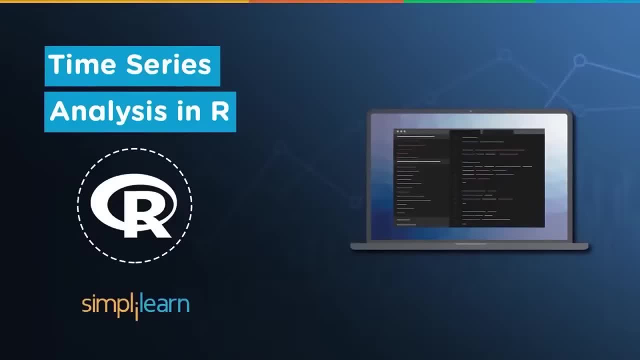 good morning and good evening everyone. so welcome to this session where we will learn on time series analysis using R programming language. so this is basically a mini project where we will look at time series data and how we can analyze it, visualize it to basically find some important information or gather insights. 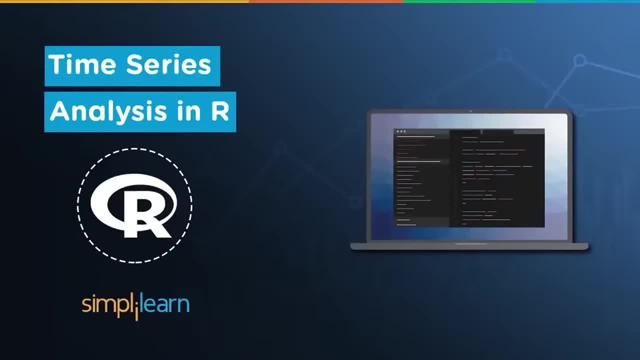 welcome to this session where we will learn on time series analysis using R programming language. so this is basically a mini project where we will look at time series data and how we can analyze it, visualize it to basically find some important information or gather insights from the data. now when? 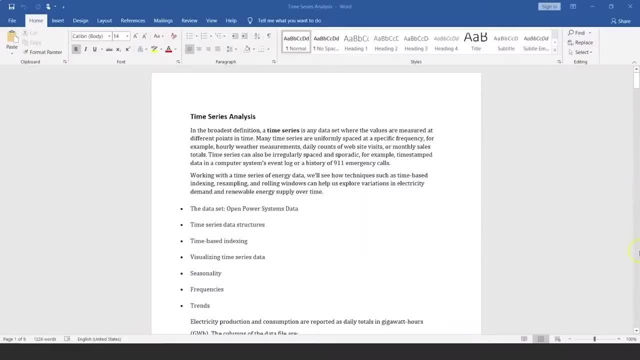 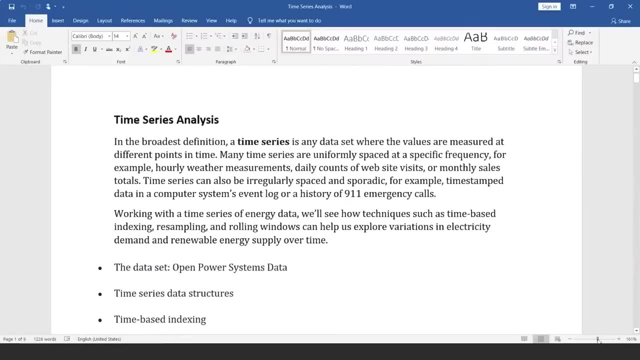 you talk about time series analysis. time series is basically any data set where your values are measured at different points in time. so when you talk about time series data, data is usually uniformly spaced at a specific frequency, for example, hourly weather measurements. you have daily counts of website visits monthly. 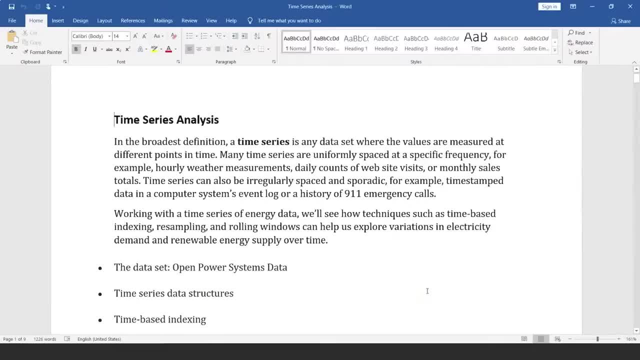 sales total and so on. so when you talk about time series, that can also be irregularly spaced and sporadic, for example, timestamp data in computer systems, event log or history of 9, 11 emergency calls. now, when we work with time series data, for example here: 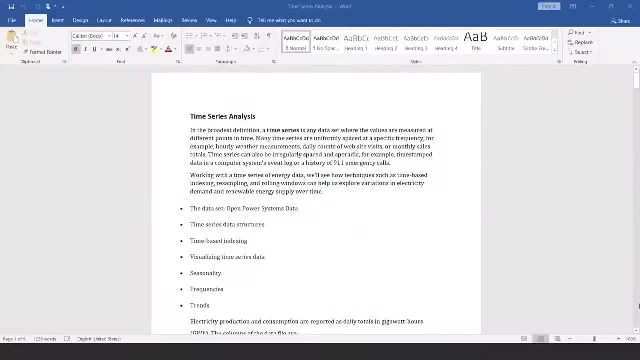 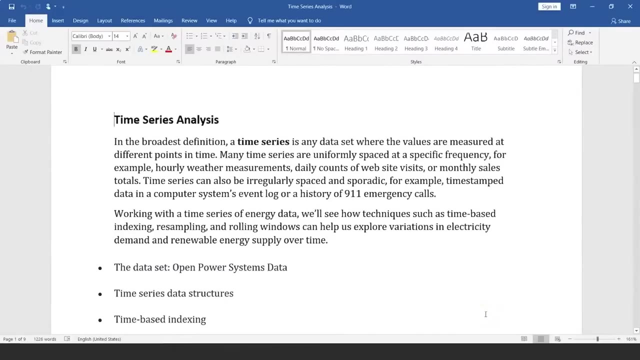 from the data. now, when you talk about time series analysis, time series is basically any data set where your values are measured at different points in time. so when you talk about time series data, data is usually uniformly spaced at a specific frequency. for example, hourly weather measurements. you have daily counts. 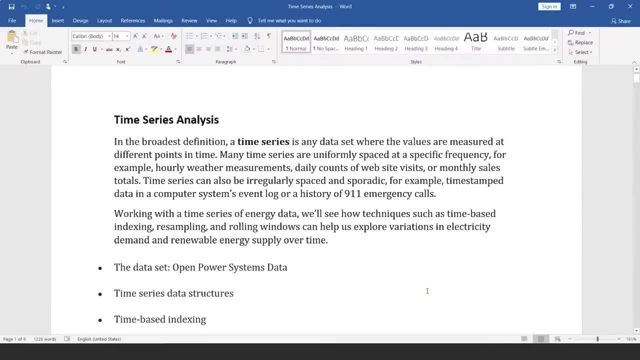 of website visits, monthly sales total and so on. so when you talk about time series, that can also be irregularly spaced and sporadic: for example, timestamp data in computer systems, event log or history of 9- 11 emergency calls. now, when we work with time series data, 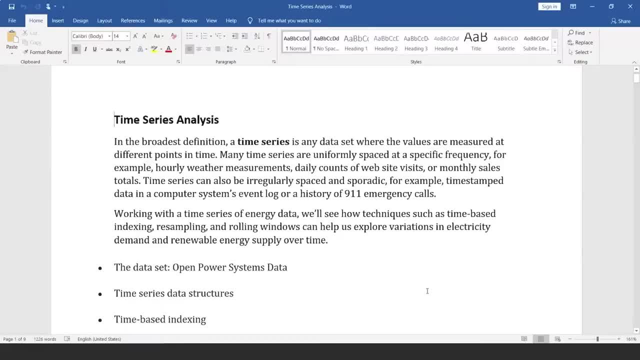 for example- here i am taking a energy data set- we can see how techniques such as time based indexing, resampling, rolling windows can help us explore variations in electricity demand and renewable energy supply over time. now here we will look at some aspects of this data set which i am considering. 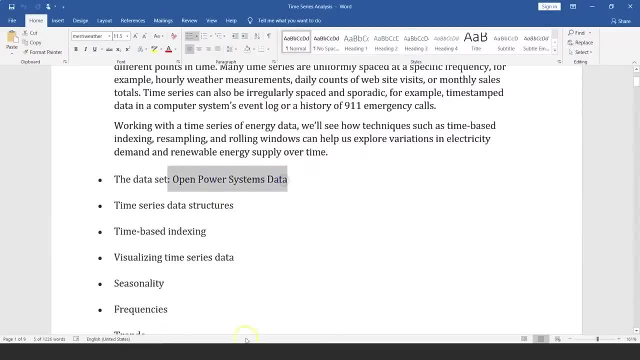 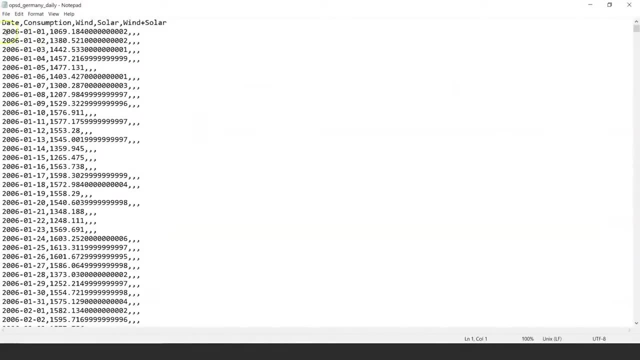 so there is- this is open power systems data set, and here is the data set i have. we can look at the data set now. this is in a simple format, it has time. it basically has values for consumption and then you have data for wind and solar and wind plus. 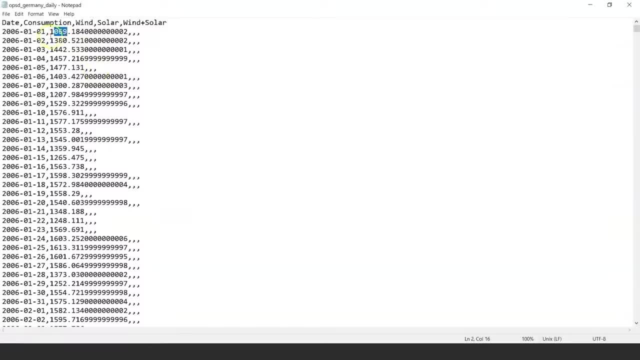 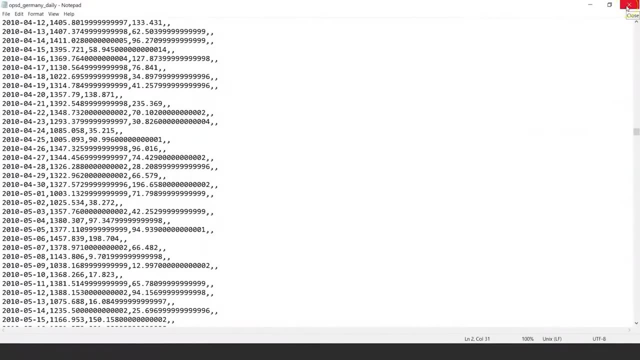 solar. so in certain cases you have only the date and the consumption, but then, if we scroll down, we will also find data for wind, solar, wind plus solar and so on. so this is a time series data set which we would want to work on. sometimes, you may. 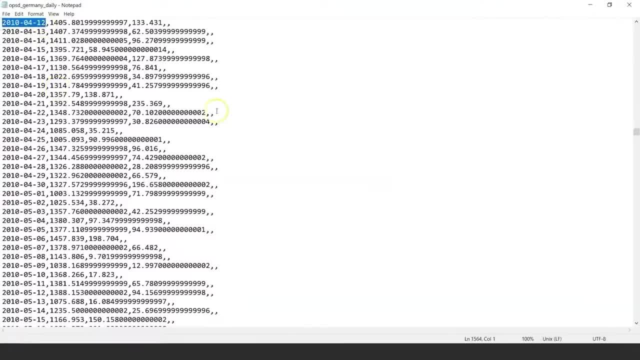 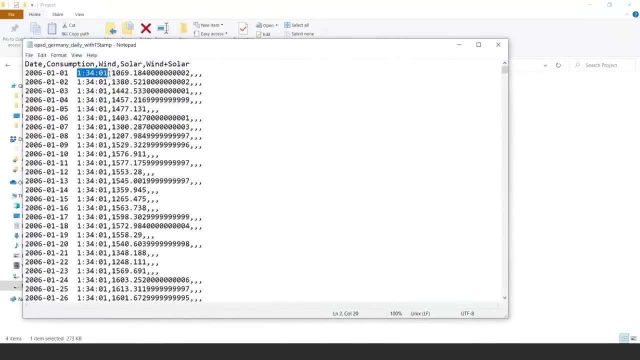 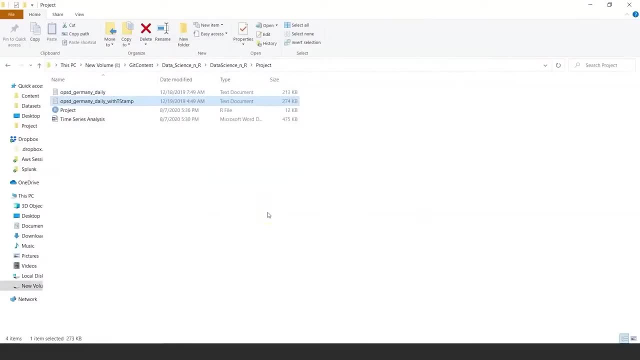 also have the data collected, which just does not have the time, but it may also have time stamp, that is, it would have, say, hour, minutes and seconds, and that can also be worked upon. so let's consider this data set and let's work on this project, where we will analyze this time. 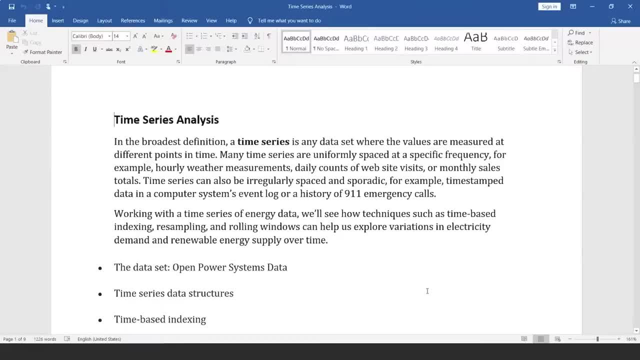 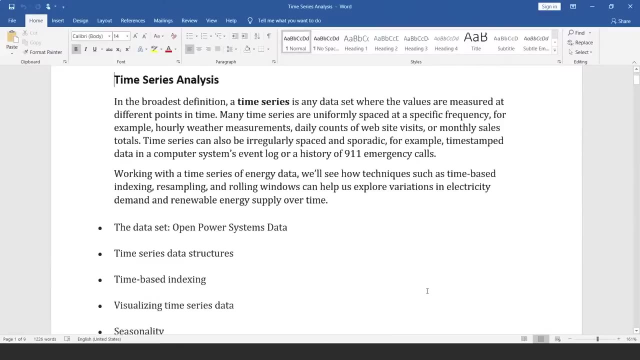 I am taking an energy data set. we can see how techniques such as time based indexing, resampling, rolling windows can help us explore variations in electricity demand and renewable energy supply over time. now here we will look at some aspects of this data set which I am considering. so there is, this is: 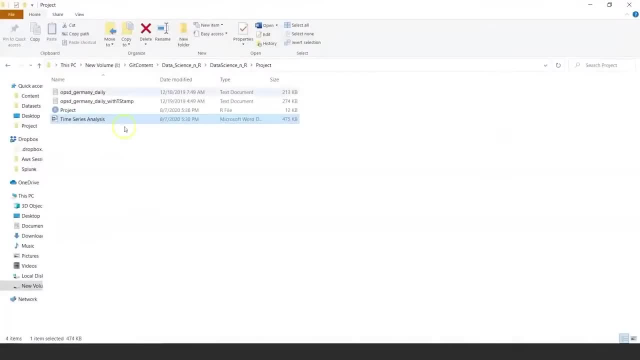 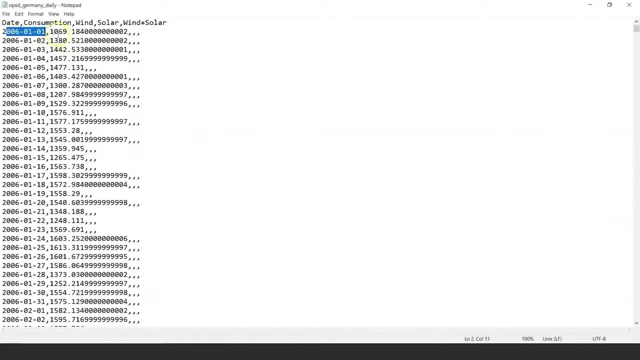 open power systems data set. and here is the data set I have. we can look at the data set now. this is in a simple format, it has time. it basically has values for consumption and then you have data for wind and solar and wind plus solar. so in certain 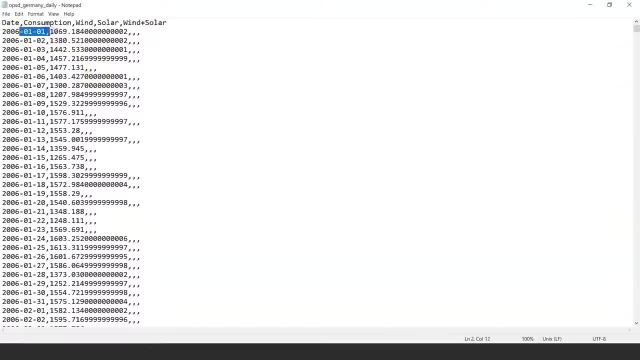 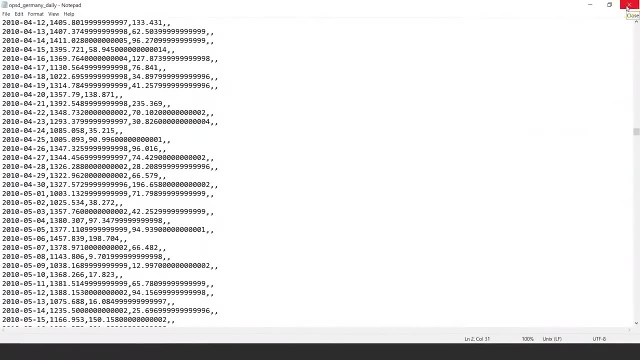 cases you have only the date and the consumption, but then if we scroll down, we will also find data for wind, solar, wind plus solar and so on. so this is a time series data set which we would want to work on. sometimes you may also have the data collected. 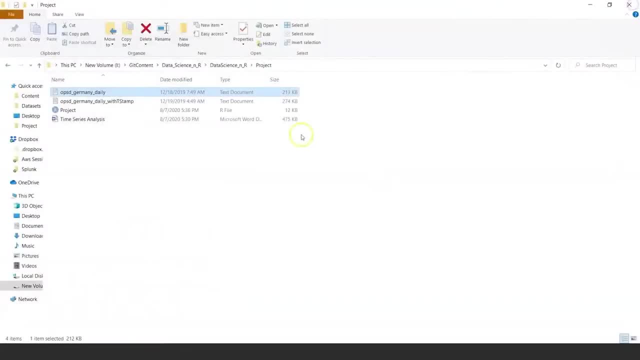 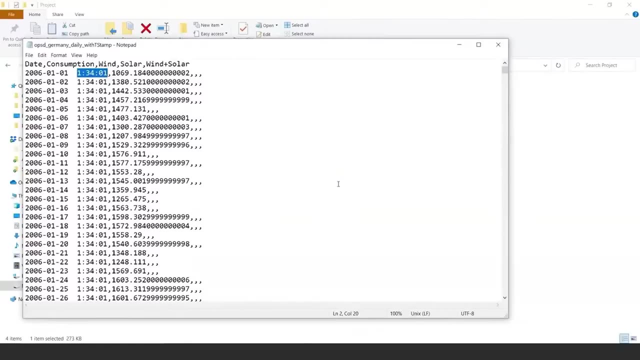 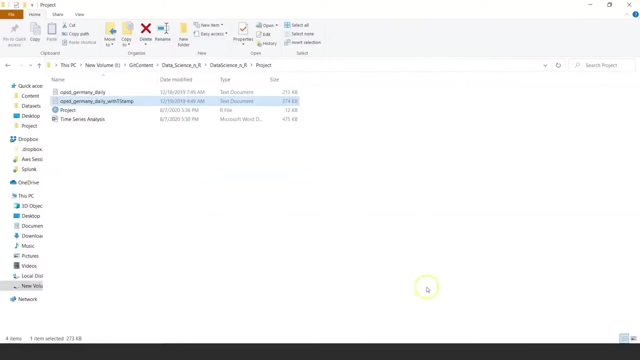 which just does not have the time, but it may also have time stamp, that is, it would have, say, hour, minutes and seconds, and that can also be worked upon. so let's consider this data set and let's work on this project, where we will analyze this time series data set. 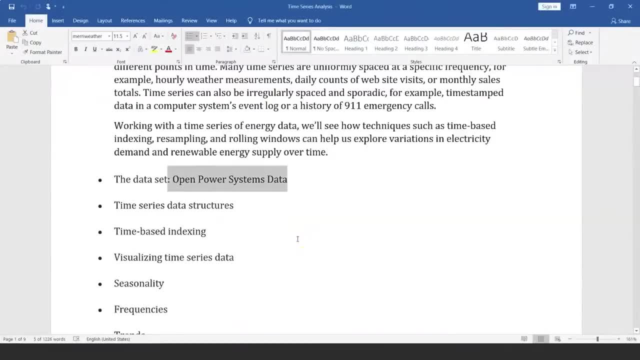 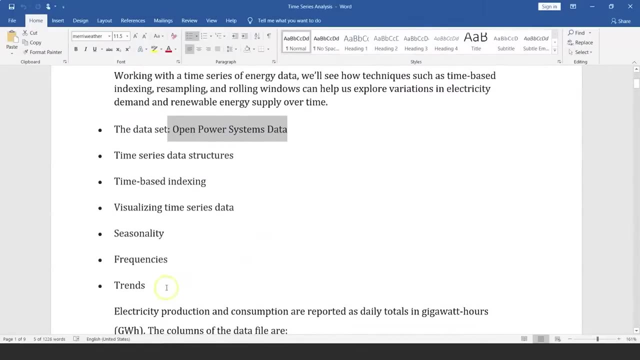 now here we can work on this time series data. we can basically create some data structures out of it, such as data frames. we can do some time based indexing. we can visualize the data. we can look at the seasonality in the data, look at some frequencies and also. 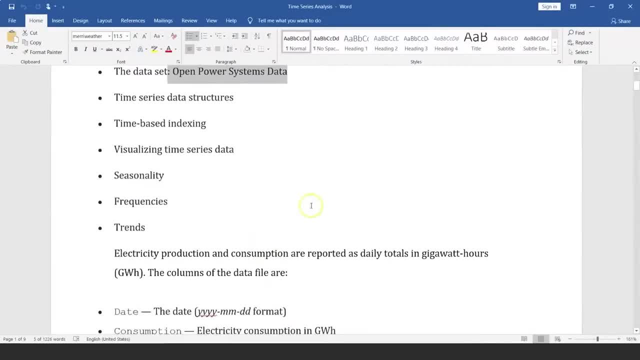 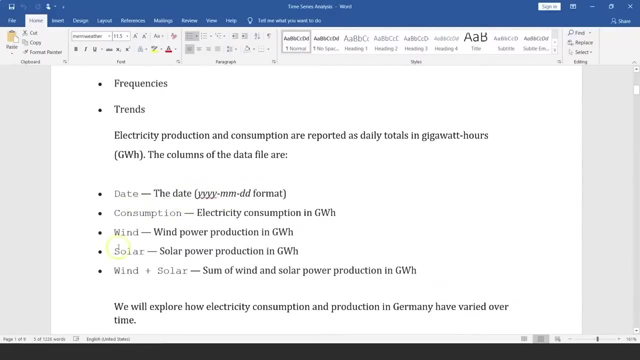 do some trend detection now. when you talk about this data set, it has electricity production and consumption which is reported as daily totals in gigawatt hours, and here are the columns of the data which I was just showing you. so you have data, you have consumption, you 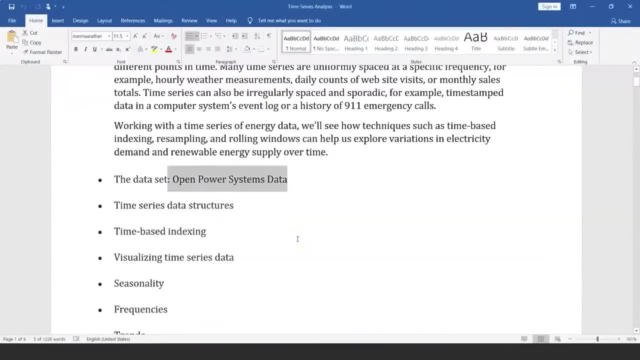 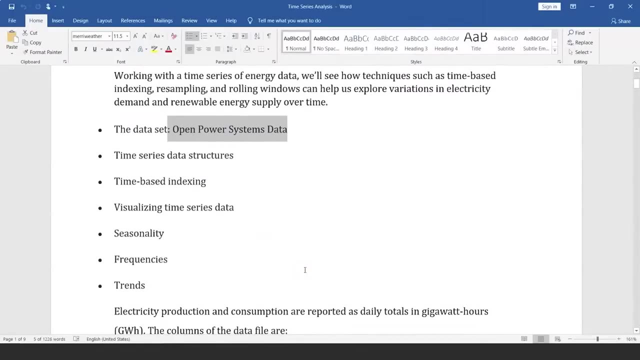 series data set. now here we can work on this time series data. we can basically create some data structures out of it, such as data frames. we can do some time based indexing. we can visualize the data, we can look at the seasonality in the data, look at some frequencies and also do. 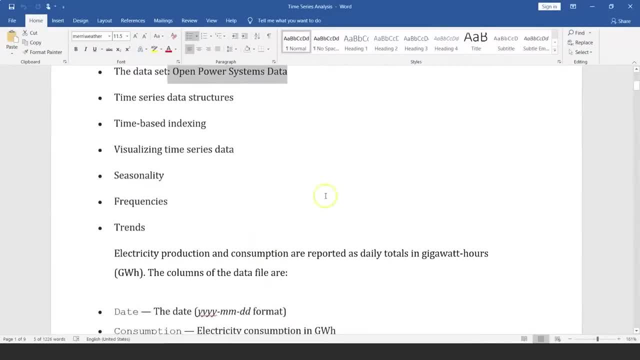 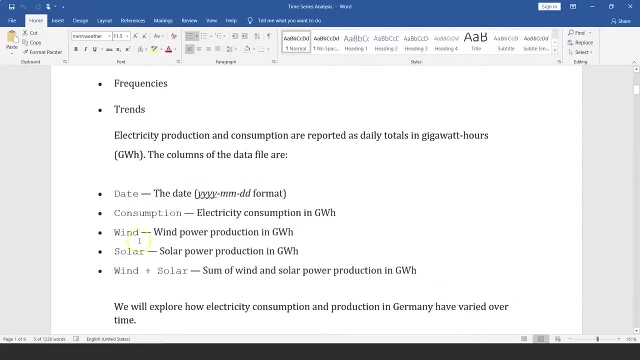 some trend detection now, when you talk about this data set, it has electricity production and consumption which is reported as daily totals in gigawatt hours, and here are the columns of the data which I was just showing you. so you have data, you have consumption, you have. 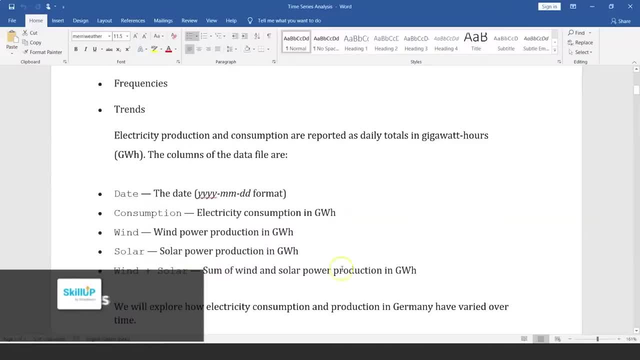 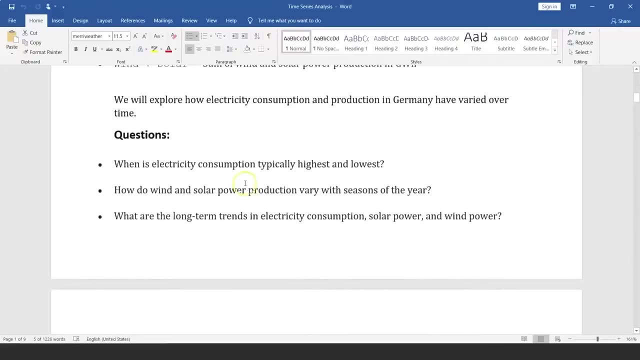 wind. you have solar and wind plus solar. so this is the data we have and we will basically explore, say, electricity consumption and production in Germany, which has varied over time. so some of the questions which we can answer here is: when is electricity consumption typically highest and lowest? 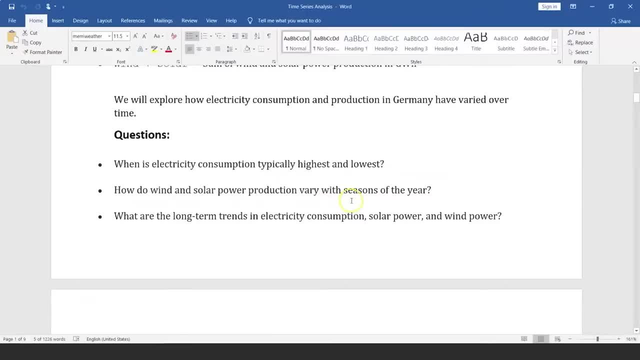 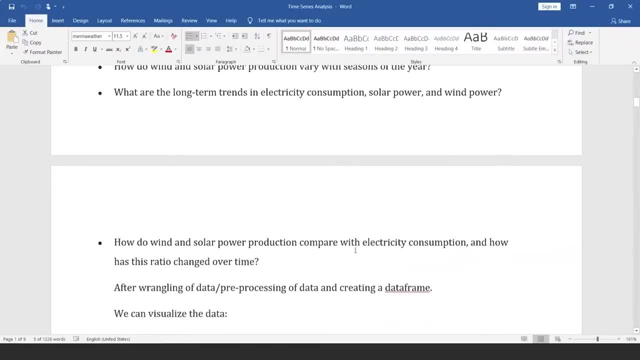 how do wind and solar power production vary with seasons of the year? what are the long term trends in electricity consumption, solar power and wind power? how do wind and solar power production compare with electricity consumption and how has this ratio changed over time? we can also do wrangling or cleaning. 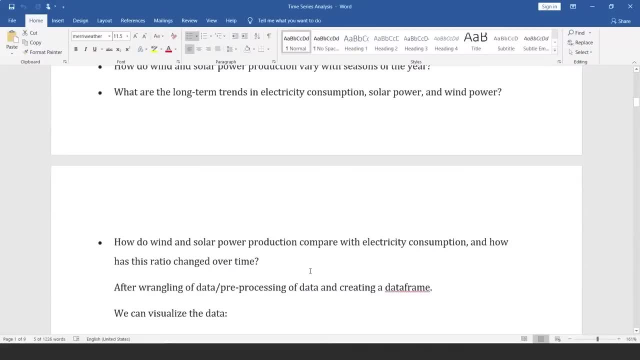 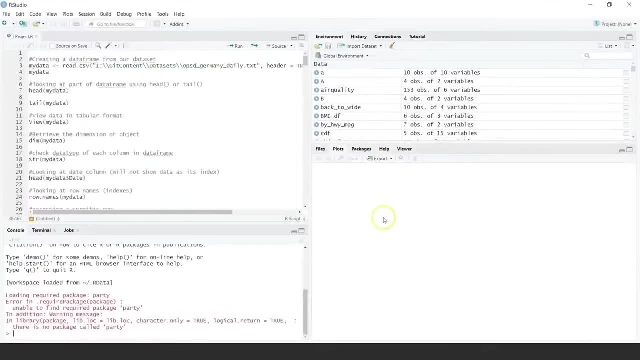 of this data, or pre-processing of data, and create a data frame, and then we can visualize this. now let's see how do we do that. so I will open up my R studio and let's look at the data set. so here is the data set. now I am. 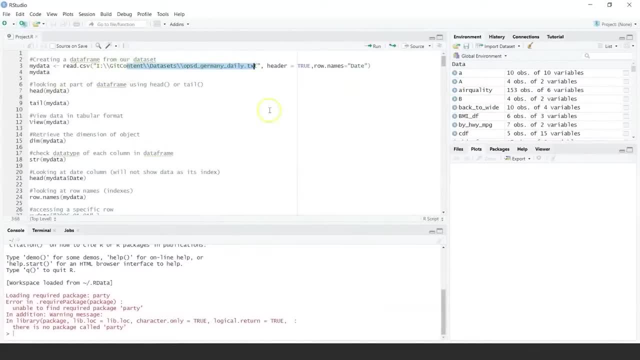 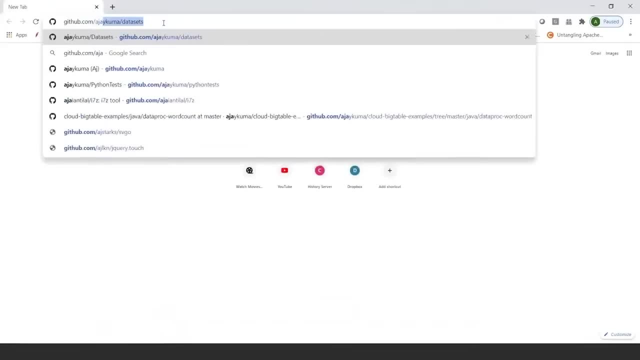 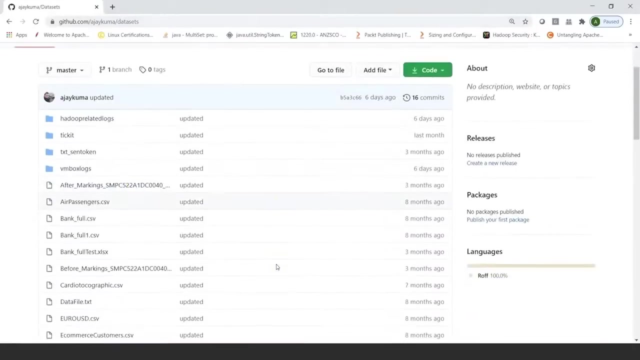 picking it up from my machine. you can also pick it up from github, so all the data sets or similar data sets can be find in my github repository and here I can look in the data sets. you will find lot of different data sets here. there are some. 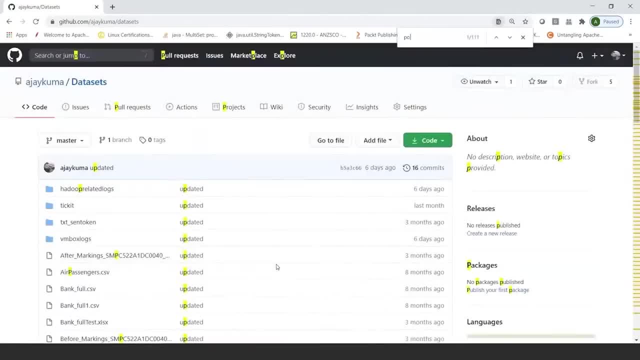 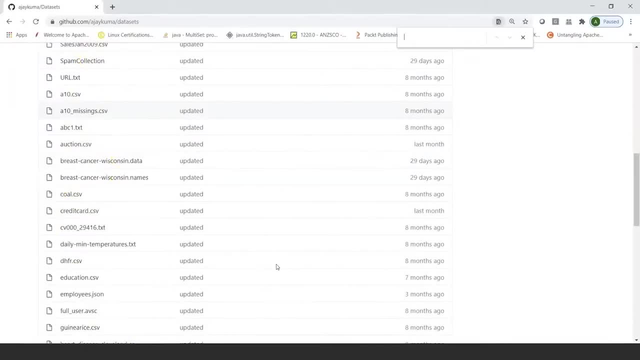 time series, data sets such as power- I can search for power, or you have basically coal, or you have this OPSD Germany daily data set and there are many other data sets which you can work on now. to get the documentation on this project, you can also look in my github repository. 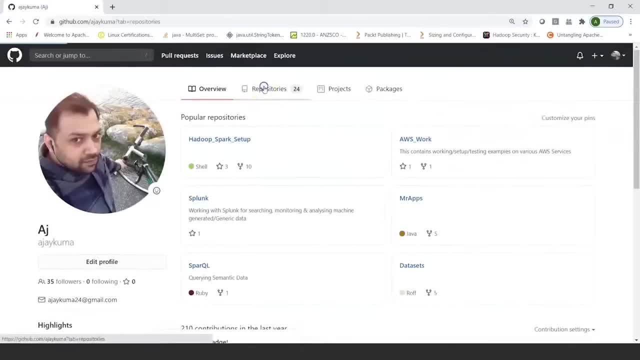 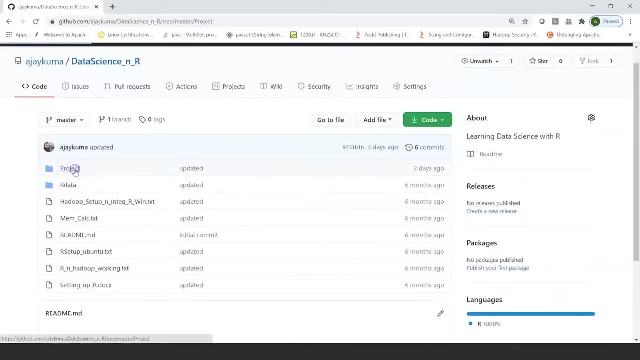 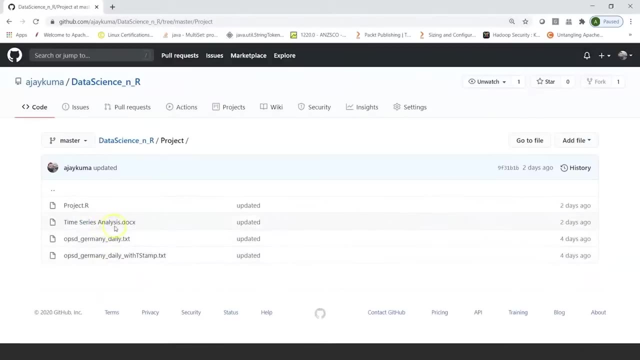 and you can search for repositories and then basically you can look in data science and R and here there is a project folder where I have given the documentation, sample data set and also your time series analysis related document. this is also the code which you can directly import in your 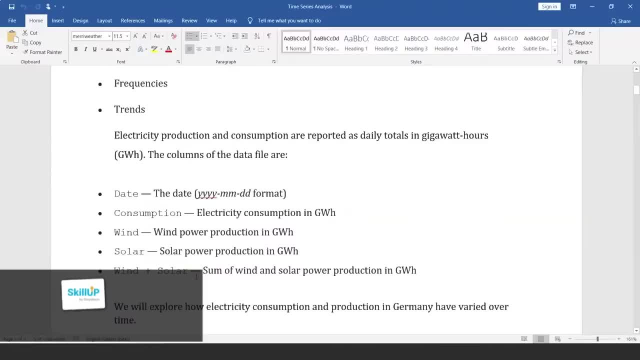 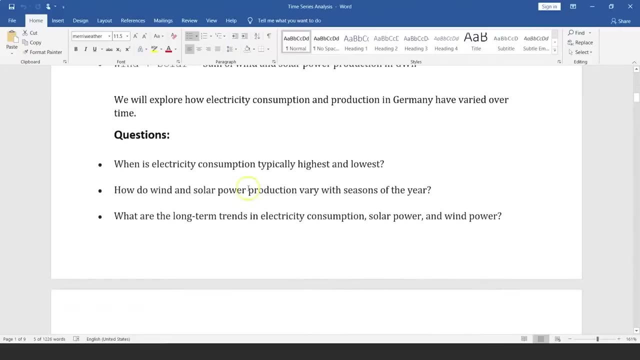 have wind, you have solar and wind plus solar. so this is the data we have and we will basically explore, say, electricity consumption and production in Germany, which has varied over time. so some of the questions which we can answer here is: when is electricity consumption typically highest and lowest? 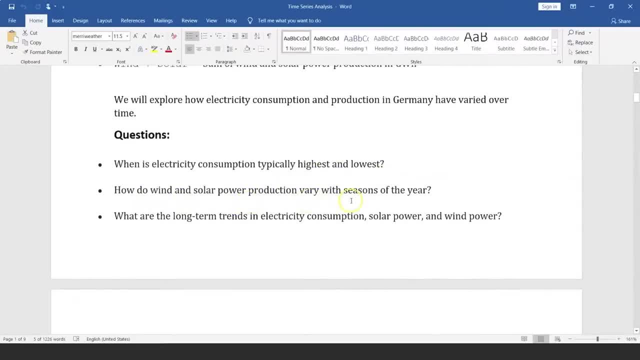 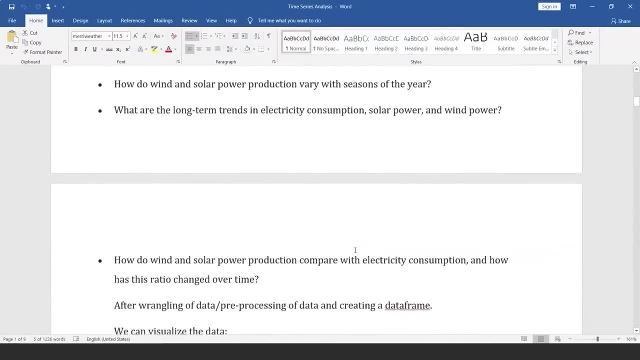 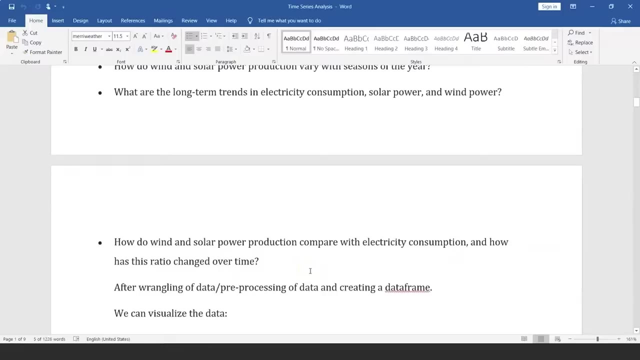 how do wind and solar power production vary with seasons of the year? what are the long term trends in electricity consumption, solar power and wind power? how do wind and solar power production compare with electricity consumption and how has this ratio changed over time? we can also do wrangling or 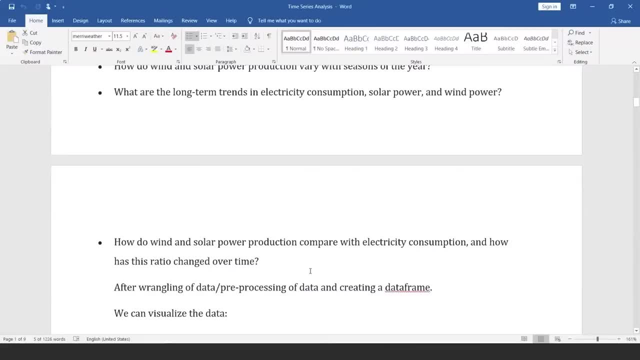 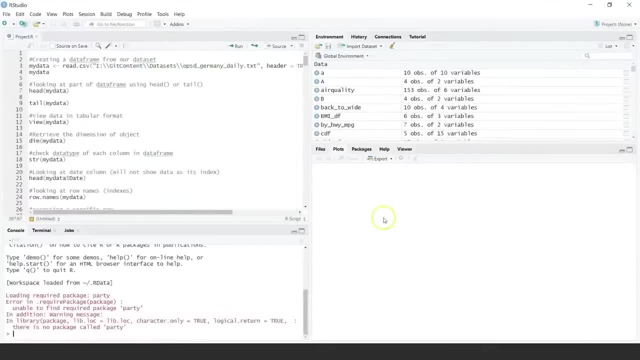 cleaning of this data or pre processing of data, and create a data frame, and then we can visualize this. now let's see how do we do that. so I will open up my R studio and let's look at the data set. so here is the data set. 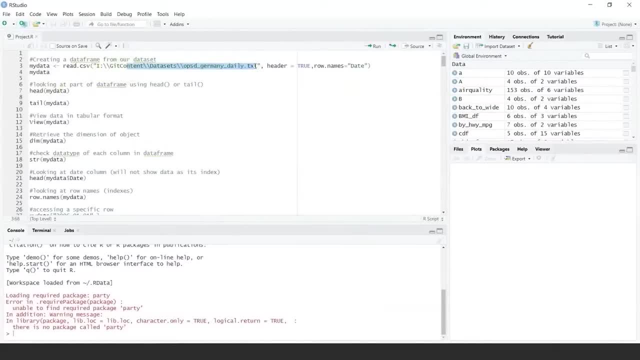 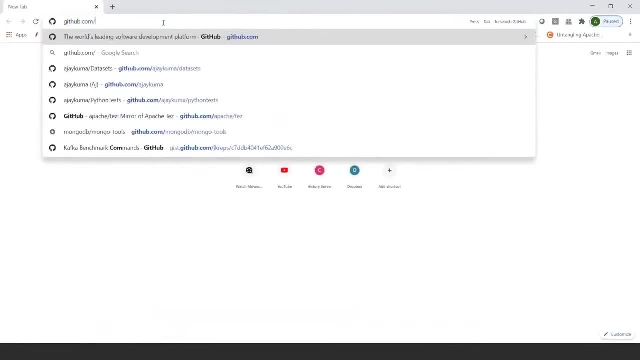 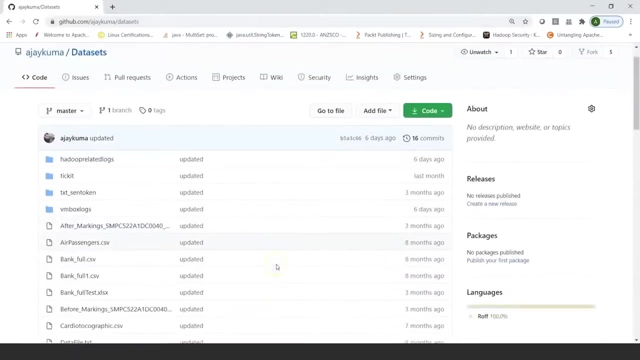 now I am picking it up from my machine. you can also pick it up from github, so all the data sets or similar data sets can be find in my github repository and here I can look in the data sets. you will find lot of different data sets here there. 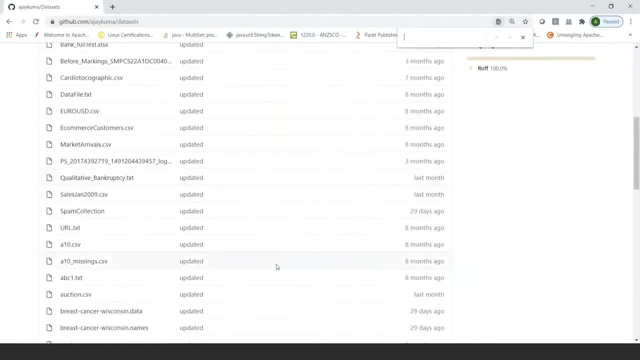 are some time series data sets such as power. I can search for power, or you have basically code or you have this OPSD Germany daily data set and there are many other data sets which you can work on now. to get the documentation on this project, you can also look in my github. 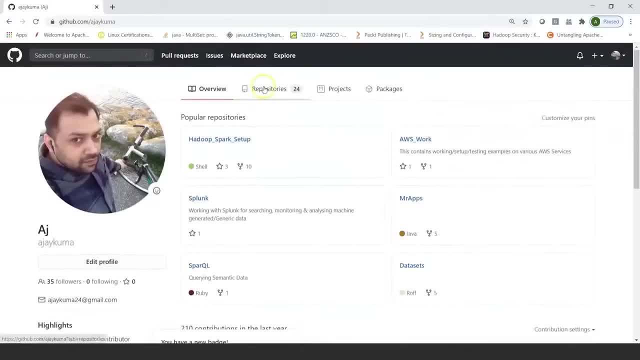 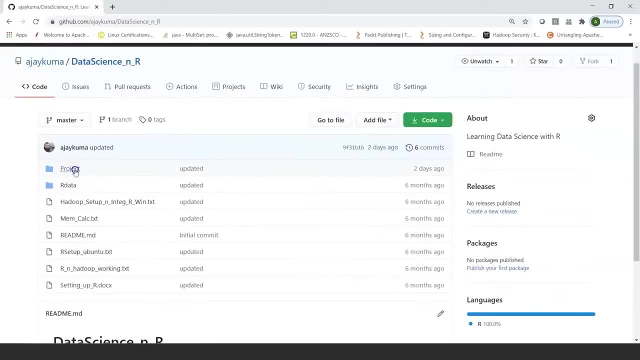 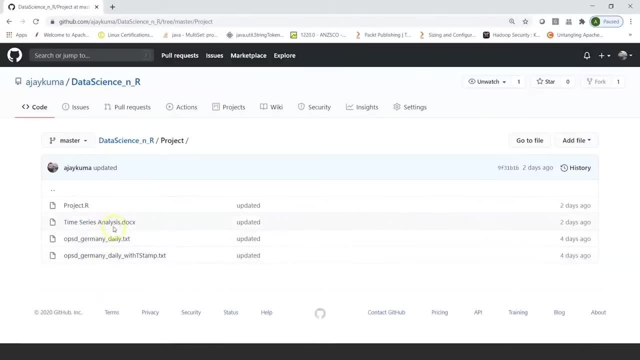 repository and you can search for repositories and then basically you can look in data science and R and here there is a project folder where I have given the documentation, sample data set and also your time series analysis related document. this is also the code which you can directly import. 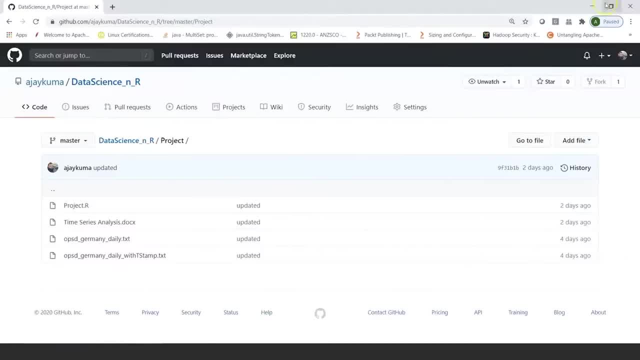 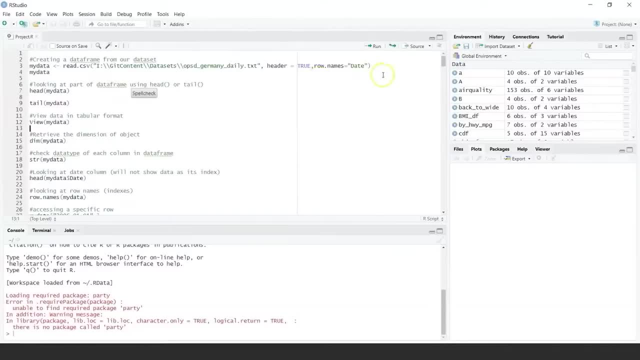 in your R studio and you can practice or work on this project. so let's see how does that work? so first thing is, we will create a data frame from this data set now here. if you see, I am using header as true so that it understands the heading. 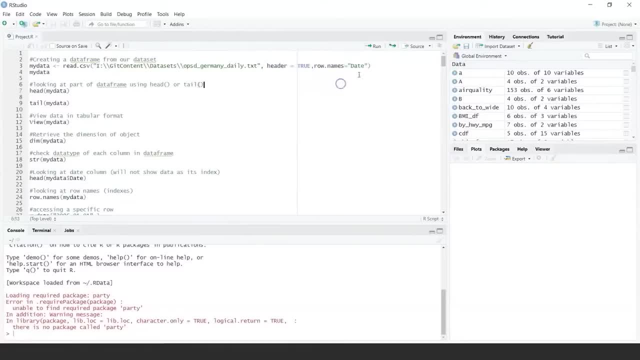 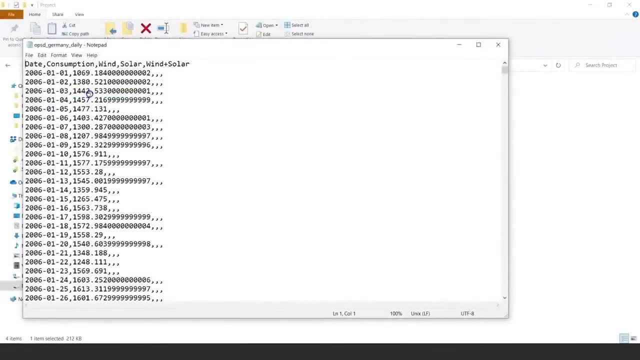 of each column. I am also giving row dot names and I am specifying date. so there is this date column in the data set, as I showed you earlier. let's look at it again. so you have date: consumption: wind, solar, wind plus solar. so you can suggest that date. 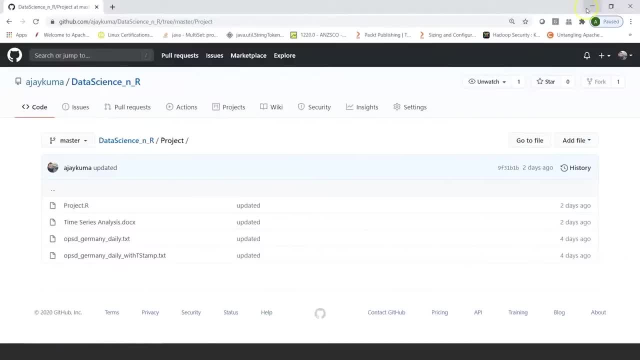 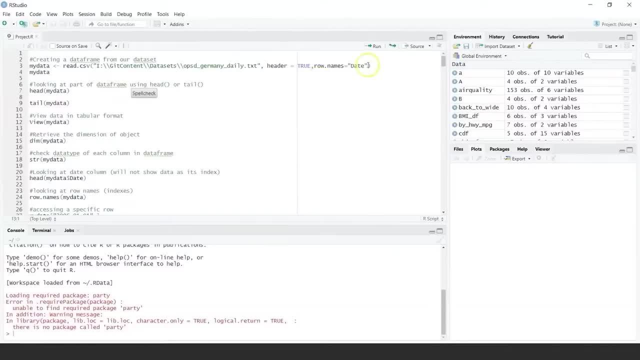 R studio and you can practice or work on this project. so let's see how does that work? so first thing is, we will create a data frame from this data set. now here, if you see, I am using header as true so that it understands the heading of: 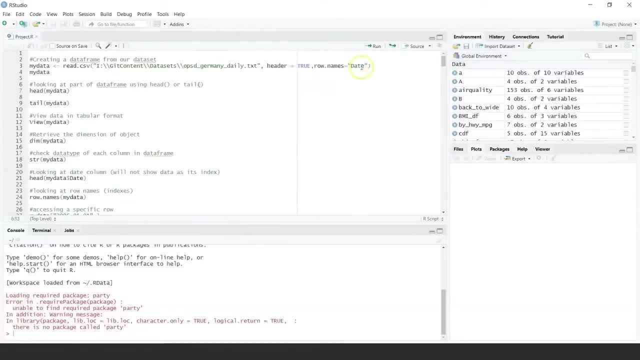 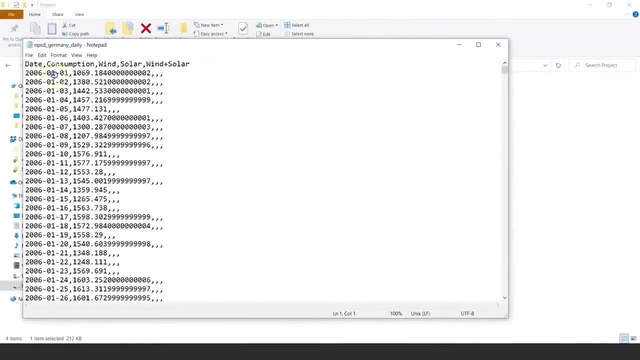 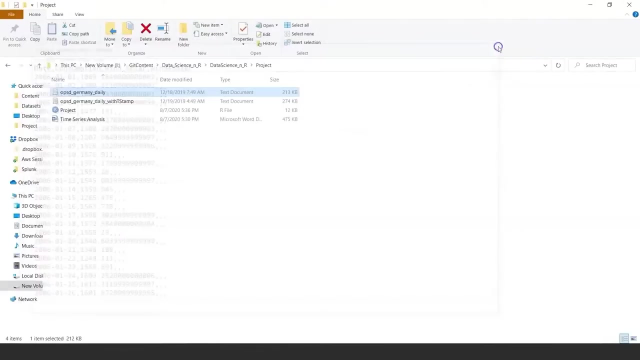 each column I am also giving row dot names and I am specifying date. so there is this date column in the data set, as I showed you earlier. let's look at it again. so you have date consumption, wind, solar, wind plus solar. so you can suggest that date should. 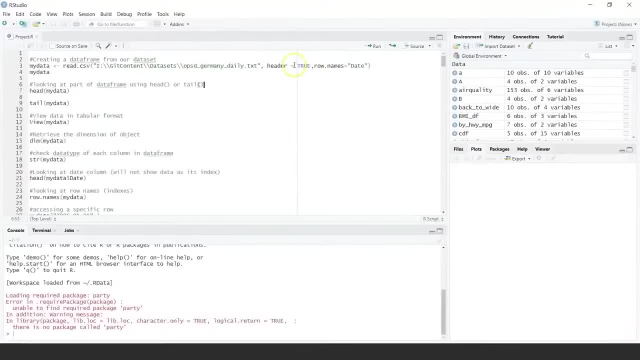 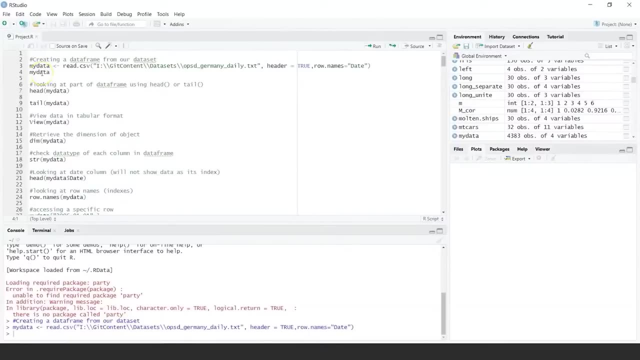 become the index column, which can be useful, so you can do this now. let's just create this. let's look at what does this data frame contain and here, if you see, it shows me some data which has been now as a part of this data frame structure. it. 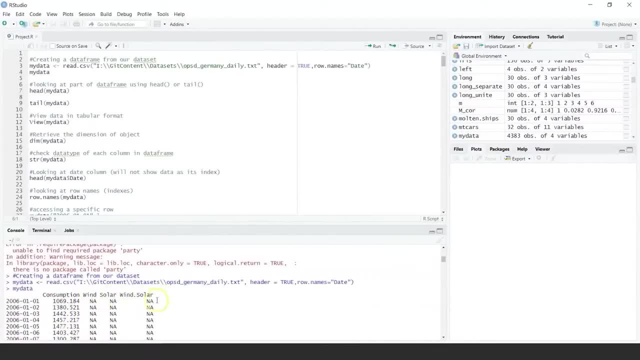 starts with consumption: wind, solar, wind plus solar. and if you see, this one is becoming my index column so I can always do a head and look at part of the data frame using head or tail. so look at the first records. so let's see this now that shows. 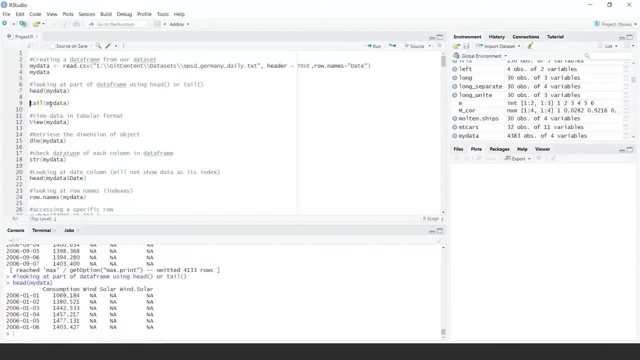 me the head data. I can also do a tail and look at the ending values. so if you closely see, here we have wind solar, wind dot solar and that basically has NA values. so there are missing values. but let's look at the tail and that tells me that there is some. 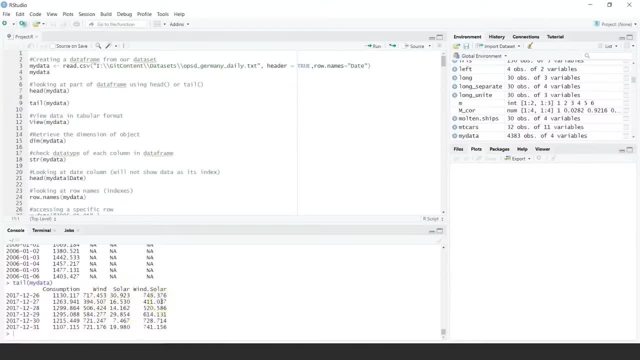 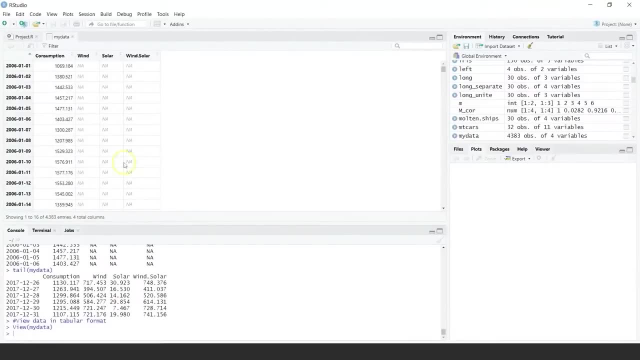 data available for wind and solar and wind solar. now we can always look in a tabular format using view and we can look at the data. so this shows me that there are values in these columns. we see NA values, but if I really scroll down I can see some values. 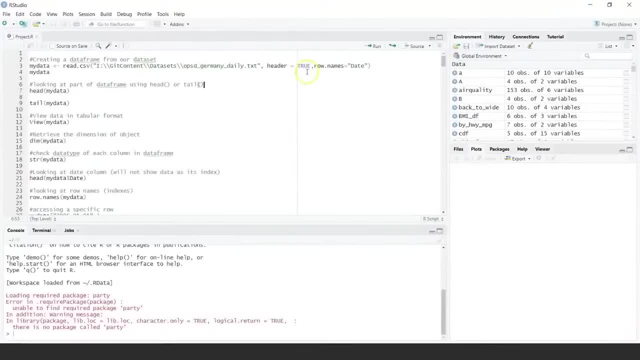 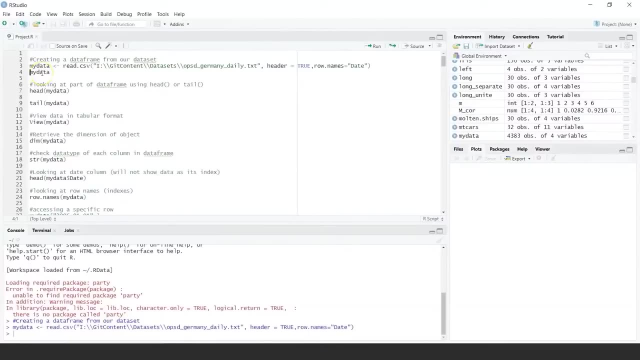 should become the index column, which can be useful, so you can do this now. let's just create this. let's look at what does this data frame contain and here, if you see, it shows me some data which has been now as a part of this data frame structure. 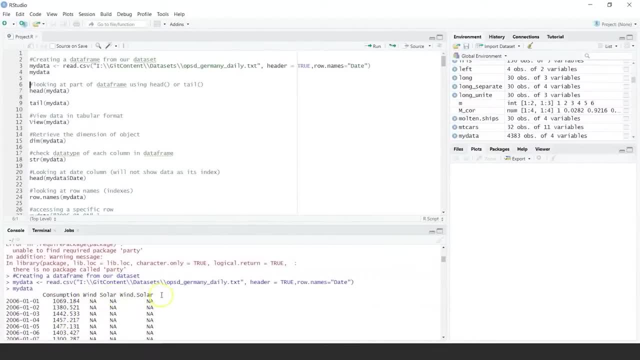 it starts with consumption: wind, solar, wind plus solar. and if you see, this one is becoming my index column so I can always do a head and look at part of the data frame using head or tail. so look at the first records. so let's see this now that 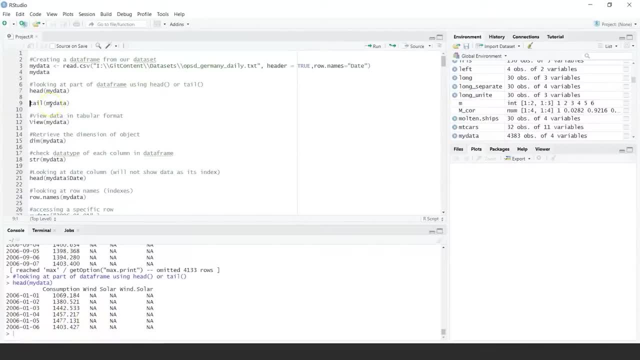 shows me the head data. I can also do a tail and look at the ending values. so if you closely see, here we have wind solar, wind dot solar and that basically has NA values. so there are missing values. but let's look at the tail and that tells me that there is. 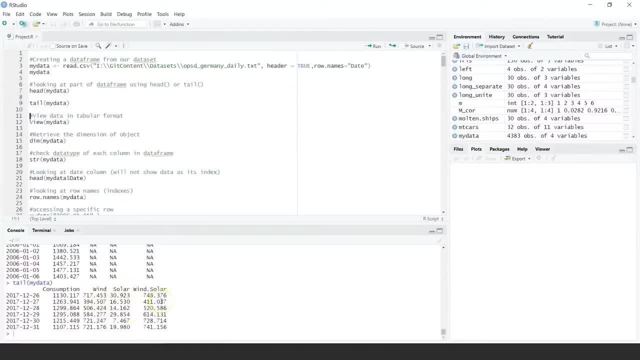 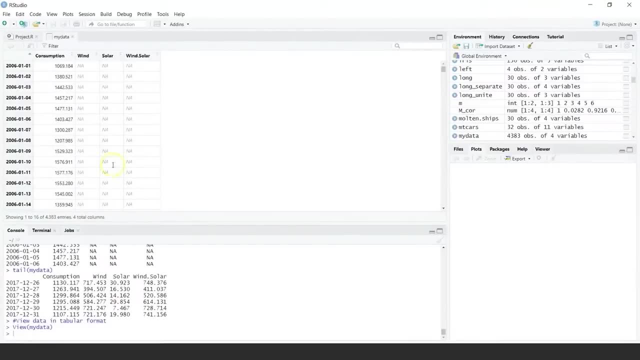 some data available for wind and solar and wind solar. now we can always look in a tabular format using view and we can look at the data. so this shows me that there are values in these columns. we see NA values, but if I really scroll down I can see some values. 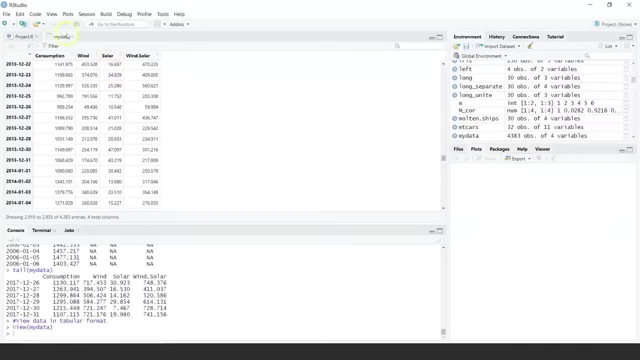 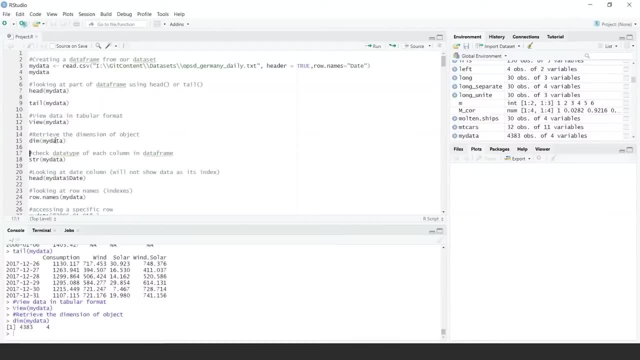 which would be available for wind and solar and wind, solar. so I can just use view. now I can look at the dimensions of this particular object and that tells me there are four hundred four thousand three hundred eighty four rows and four columns. you can always look at the structure. that is check. 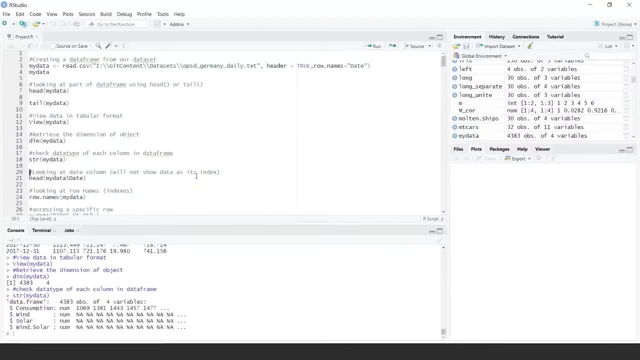 the data type of each column, which can be very useful. so if I see here, I don't see the date column, because date column was considered as an index which can be useful. but I also look at my other columns, they are of the num types, so that's the data type for each. 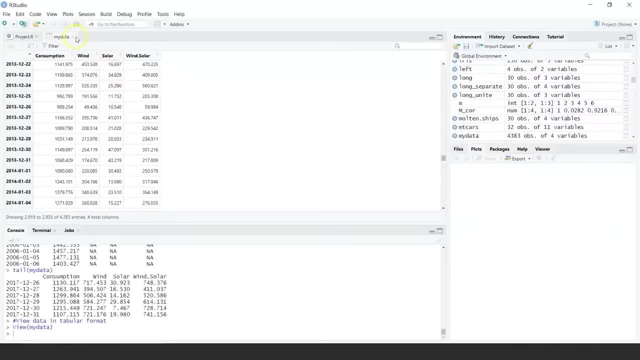 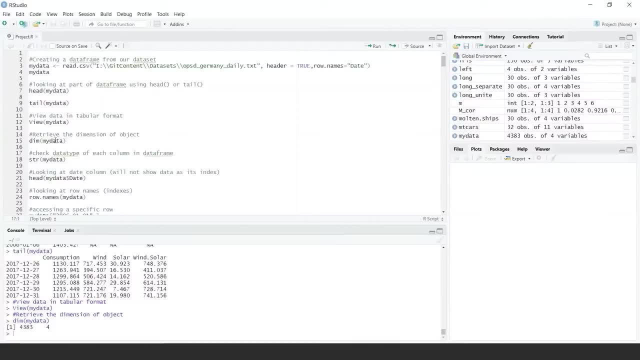 which would be available for wind and solar and wind, solar. so I can just use view. now I can look at the dimensions of this particular object and that tells me there are 4384 rows and 4 columns. you can always look at the structure, that is, check the data. 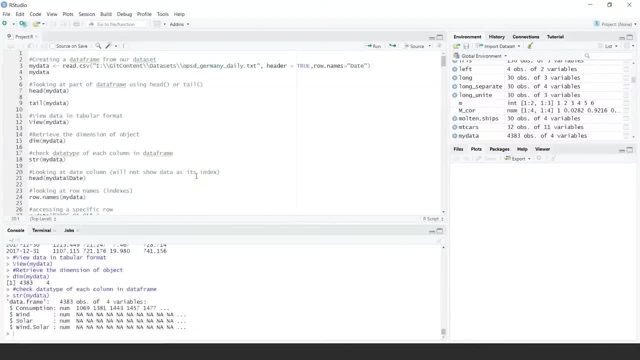 type of each column which can be very useful. so if I see here, I don't see the date column, because date column was considered as an index which can be useful. but I also look at my other columns, they are of the num types, so that's the data type for each and 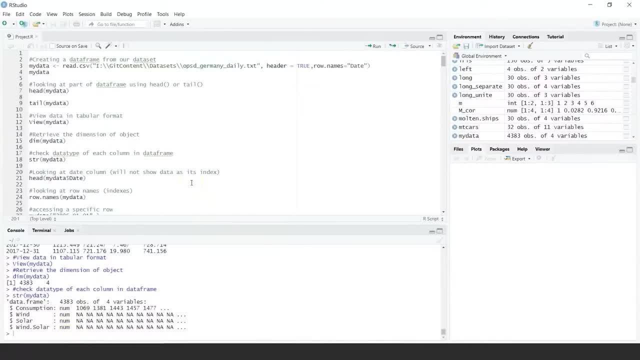 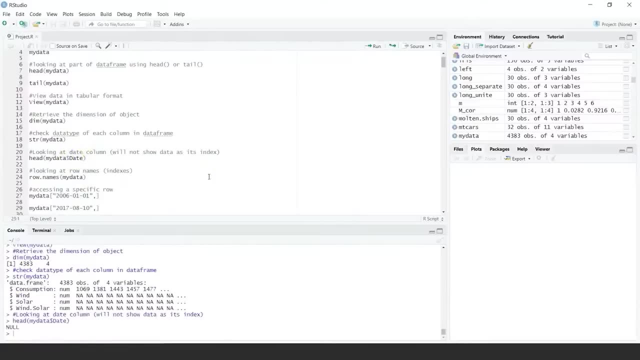 attribute or each column here now we would be interested in looking at this date column. so let's look at the data type of this date column now. if I try to do this, this will show me that this is null, because date as a column does not exist, because we created 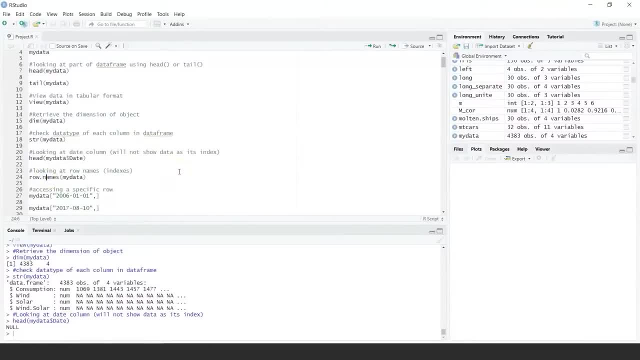 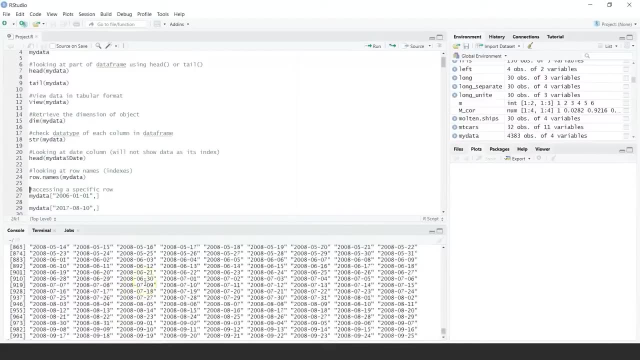 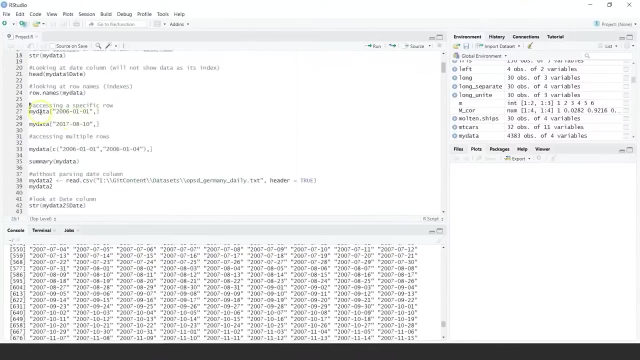 it as an index. so if I look at row names and then I search for my data, show me the index column or rownames, it tells me these are the values. that's the date column which we are seeing here now. we can access a specific row by just. 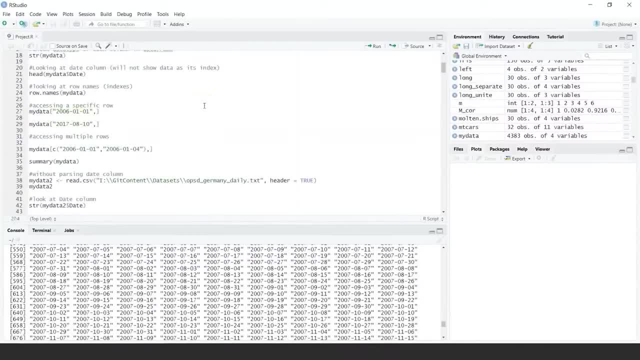 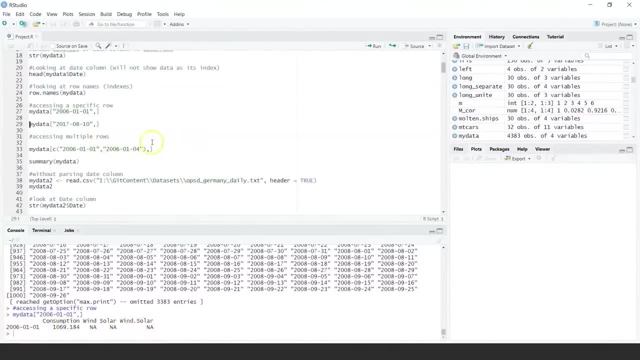 doing a my data and give the index value or row name value. so let's look at that and that shows me. based on this index, you are looking at the value. you can obviously search for a different date, something like this. you can also pass in a vector and you can. 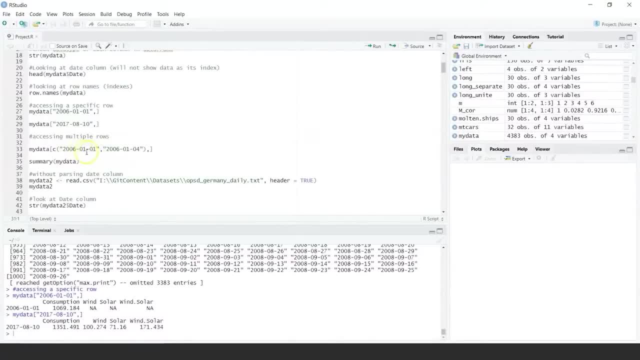 give range of values. so that is 0: 1, 2006 to 4 of January, and we can look at this one so it shows me these are the values. so here, actually, I am not giving a range, but I am just selecting multiple values from rownames. 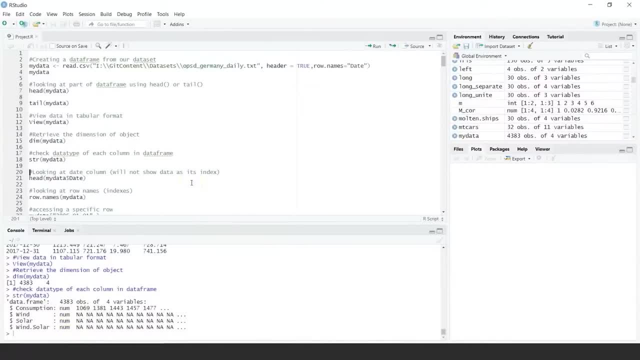 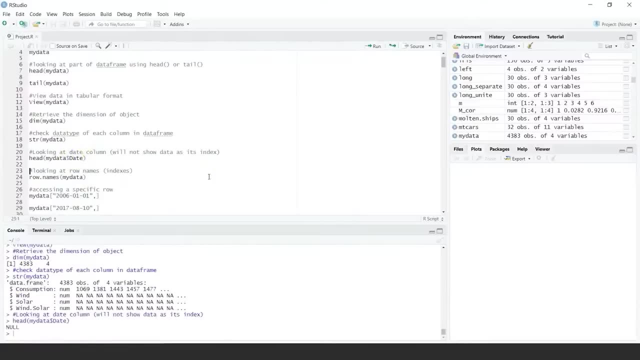 attribute or each column here now we would be interested in looking at this date column. so let's look at the data type of this date column now. if I try to do this, this will show me that this is null, because date as a column does not exist, because 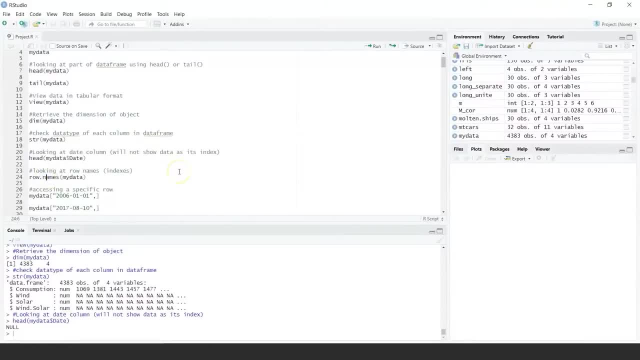 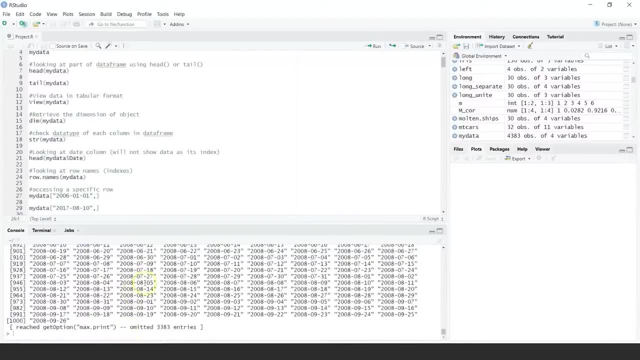 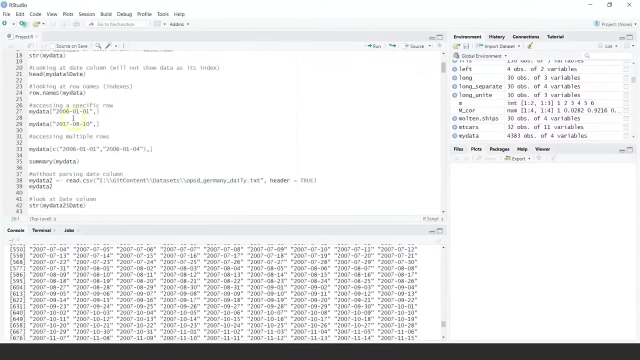 we created it as an index. so if I look at row names and then I search for my data, show me the index column or row dot names, it tells me these are the values, that's the date column which we are seeing here. now we can access a specific row. 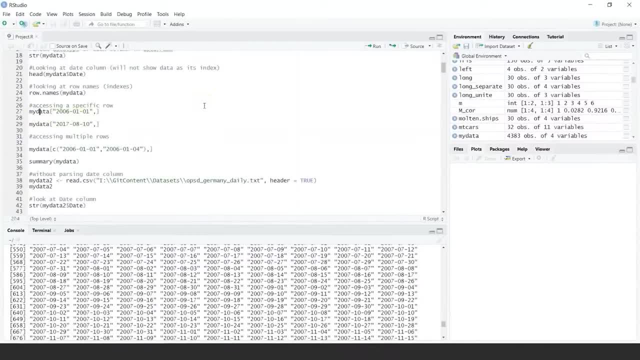 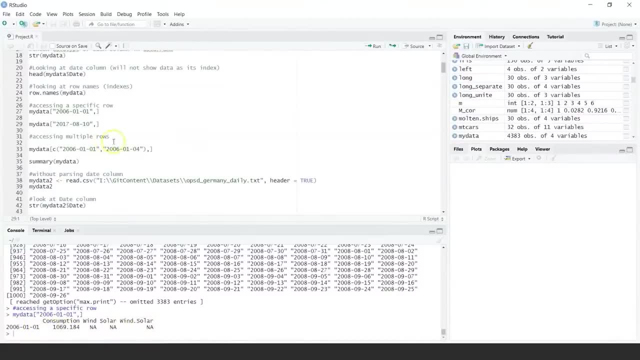 by just doing a my data and give the index value or row name value. so let's look at that and that shows me. based on this index, you are looking at the value. you can obviously search for a different date, something like this: you can also pass in a vector and: 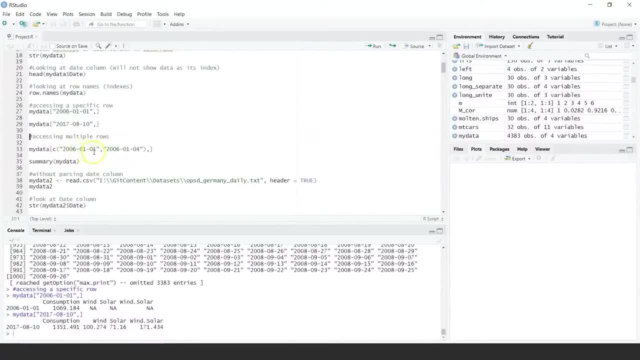 you can give range of values. so that is 0: 1 2006 to 4 of January, and we can look at this one. so it shows me these are the values. so here, actually, I am not giving a range, but I am just selecting multiple values from 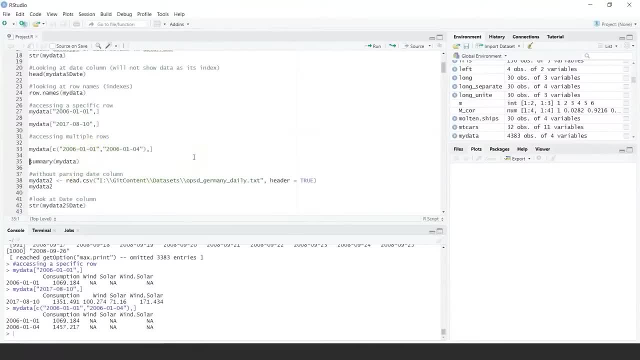 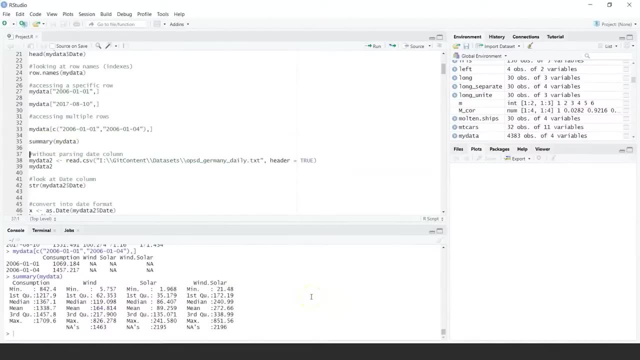 row dot names. now we already know that in R you have a summary function, so you can always do a summary and that gives you for each column. it gives you minimum, first quartile, median mean, third quartile and maximum values. so we are looking at consumption, we are looking at wind, solar. 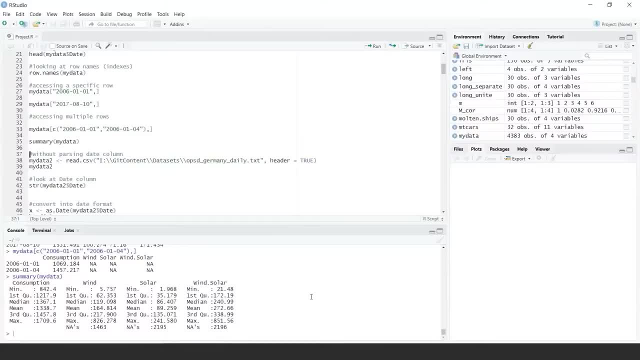 and wind, dot, solar. now this is good. but then if I would want to really visualize the data, access the data, do some analysis, then it would be good to take all the columns and then we can later decide to change the data type of, say, date column. if 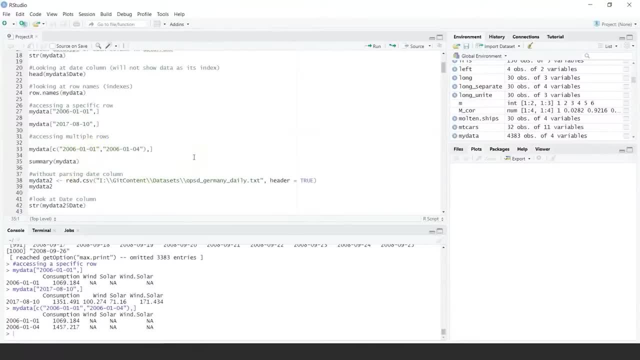 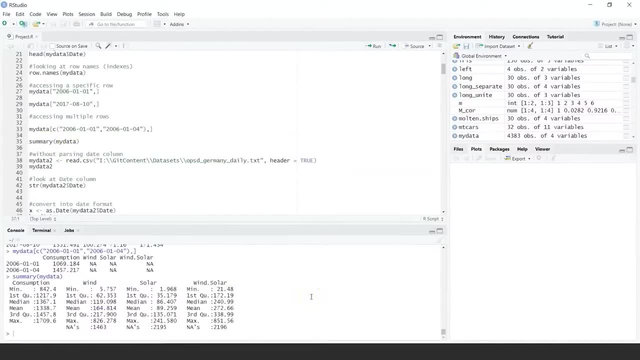 now we already know that in R you have a summary function, so you can always do a summary and that gives you for each column. it gives you minimum, first quartile, median mean, third quartile and maximum values. so we are looking at consumption, we are looking at wind- solar and wind. 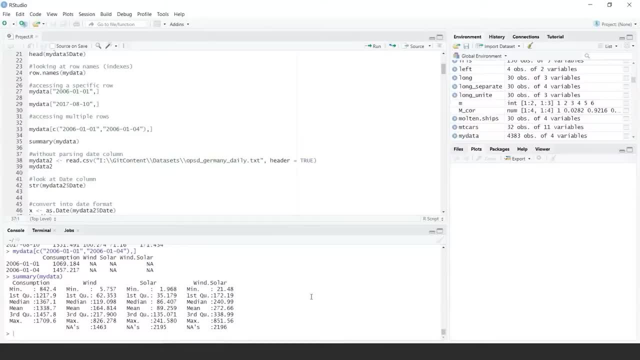 dot solar. now this is good, but then if I would want to really visualize the data, access the data, do some analysis, then it would be good to take all the columns and then we can later decide to change the data type of, say, date column if we want. 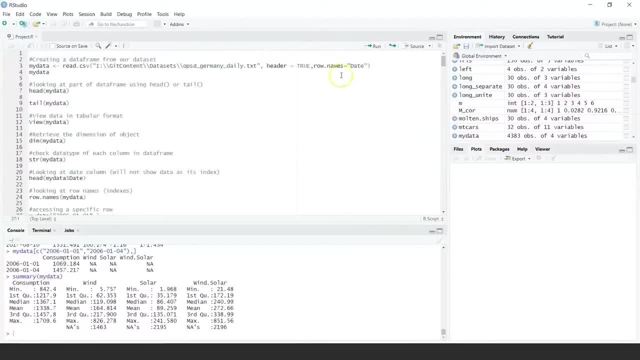 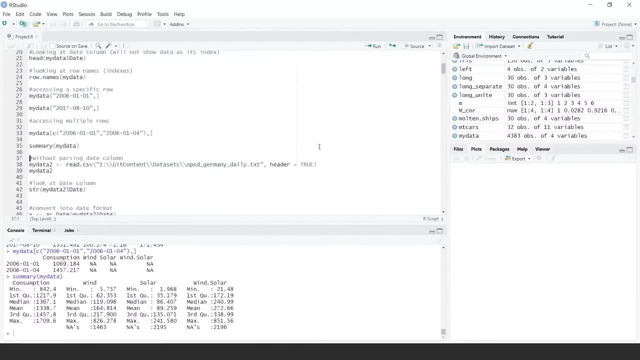 we want to use it. so earlier I was using date as row dot names or the name of the rows, or index, what you call in any other programming language. so here I will just use my data set and I will say header: is true, I am calling it my data. 2. let's 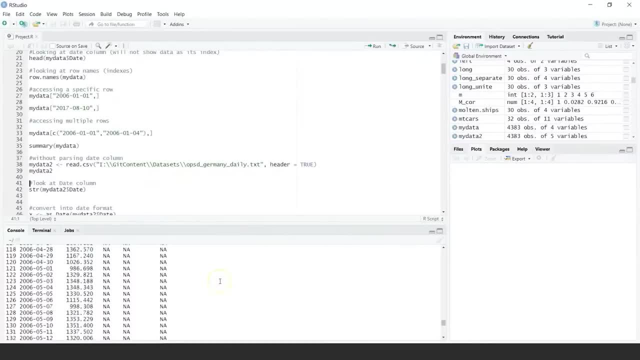 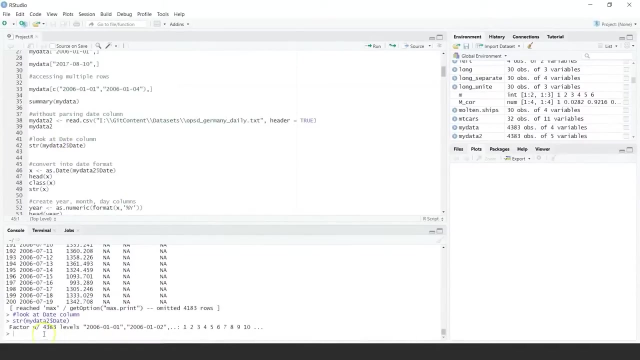 look at the data, and this one shows me 5 columns, where in my first column is the date: consumption: wind, solar and so on. now looking at the structure. so let's look at the data type. so it tells me that if now I am interested in looking at the date column, 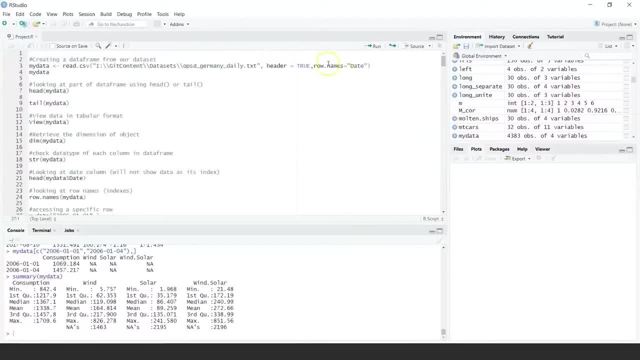 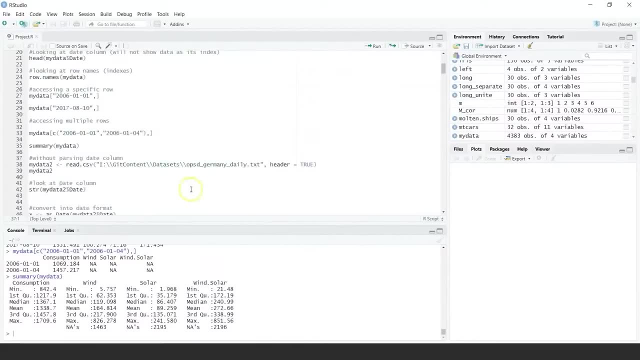 to use it. so earlier I was using date as rownames, or the name of the rows, or index, what you call in any other programming language. so here I will just use my data set and I will say: header is true, I am calling it my data 2. let's look at: 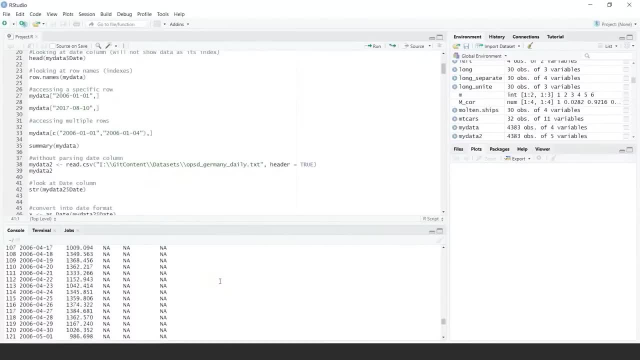 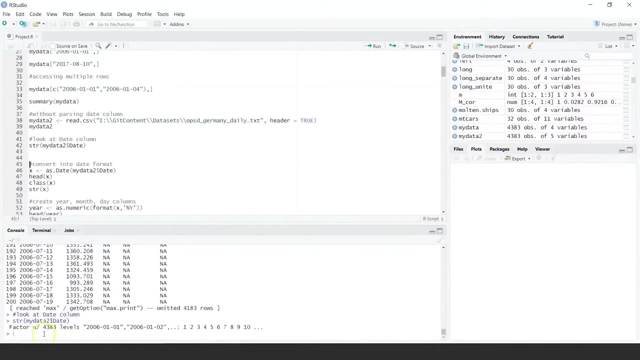 the data, and this one shows me 5 columns, where in my first column is the date: consumption: wind, solar and so on. now looking at the structure. so let's look at the data type. so it tells me that if now I am interested in looking at the date column, 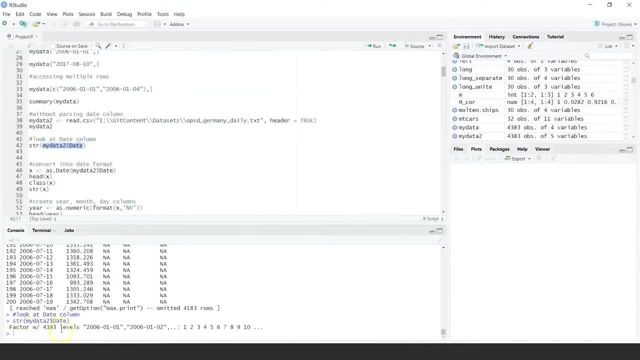 from my data 2 data frame. it tells me it is a factor with 4384 levels and these are the values. so it is not in a date time format, it is a factor. now what we can do is we can convert this into a date format. 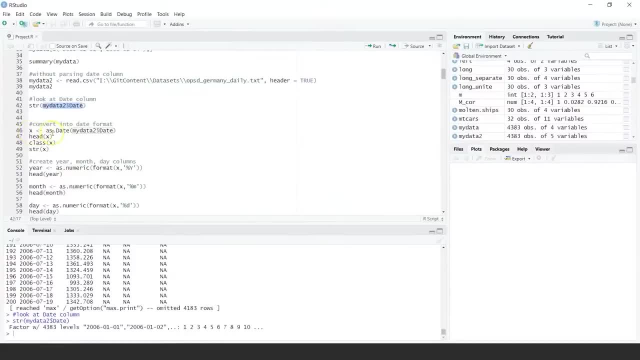 how do we do that? so let's have a variable x and I am going to use as dot date function and I am going to pass in my date column, so that's assigned to x. now let's look at the header of x and it shows me the values. 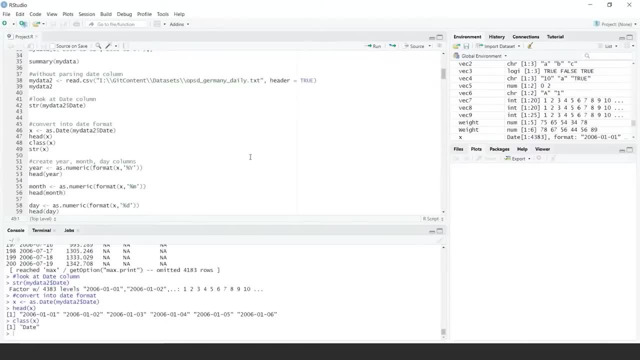 we will also see what kind of class it is and we will look at the structure of x. so class already says it is date type and look at the structure. so it shows me the format. now we have converted this column or column related value into x. now how do I? 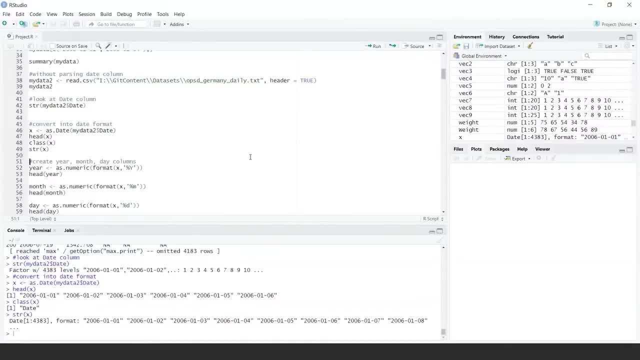 basically extract values out of it or make it a part of data frame. so first I will use so all. once it has been converted in data format, I will go for as dot numeric and here I will create a variable called year and I will just do a format on. 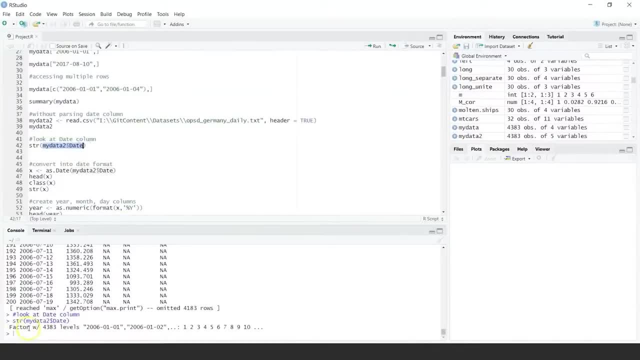 from my data 2 data frame. it tells me it is a factor with 4384 levels, and these are the values. so it is not in a date time format, it is a factor. now what we can do is we can convert this into a date format. how do we do that? so 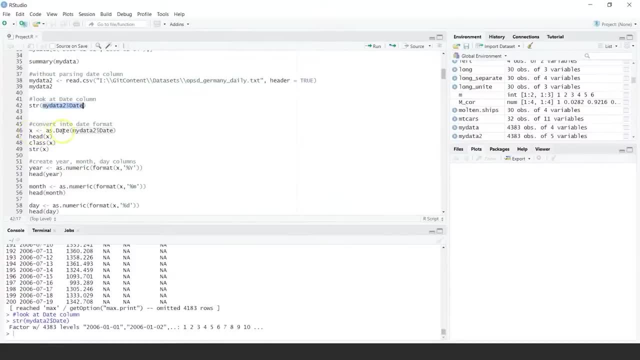 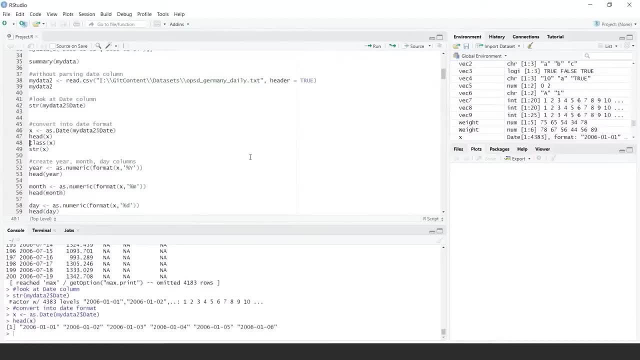 let's have a variable x and I am going to use as dot date function and I am going to pass in my date column so that's assigned to x. now let's look at the head of x and it shows me the values. we will also see what kind. 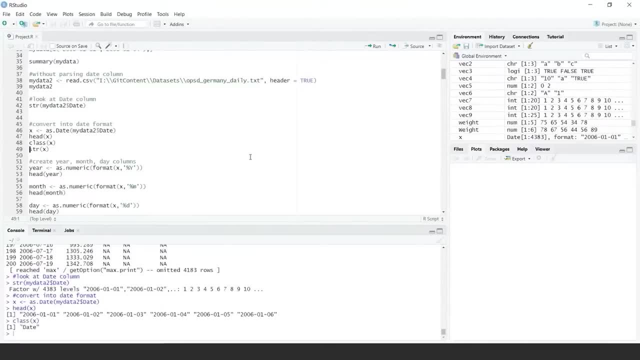 of class. it is and we will look at the structure of x. so class already says it is date type and look at the structure. so it shows me the format. now we have converted this column or column related value into x. now how do I basically extract values out of it or make it? 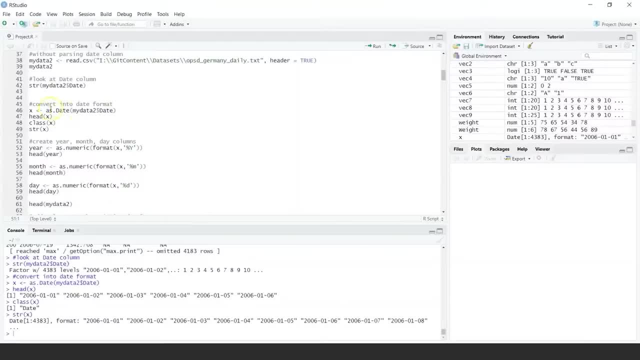 a part of data frame. so first I will use so all. once it has been converted in date format, I will go for as dot numeric and here I will create a variable called year, and I will just do a format on x, which is basically of date type. and then I am saying: 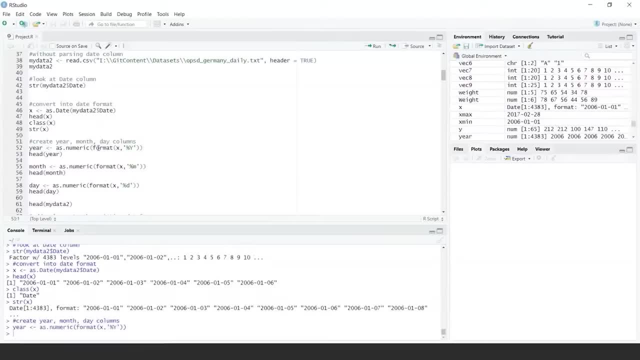 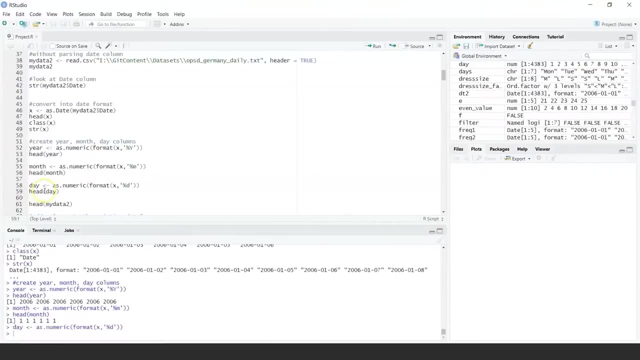 %y. so that will get me the year component out of this. let's look at the values. that shows me year component. now, similarly, we can get the month out of this and then basically look at the month values. we can get the day out of it and we can get the. 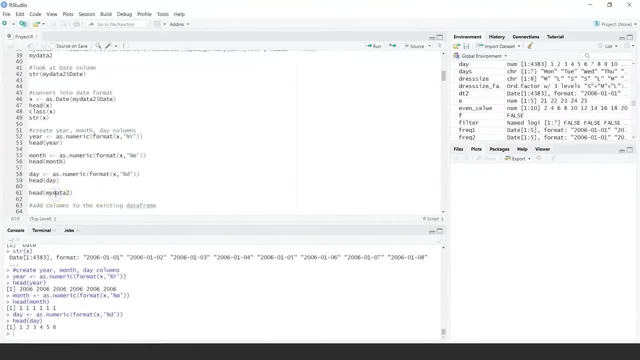 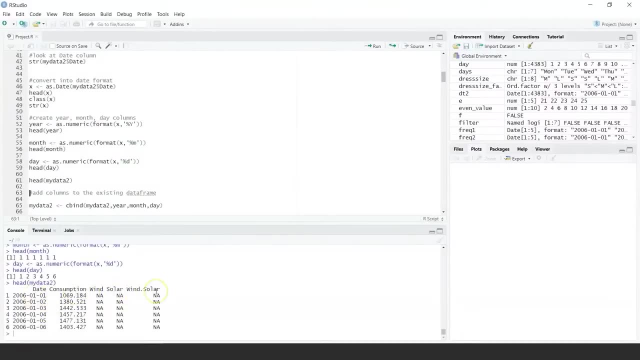 day component. now, if I look at my data 2, which we had created earlier, this basically had date consumption: wind solar, wind solar. so what I can do is I can add these extracted columns, such as year, month, day, to my data frame using a c bind, that is, column bind. 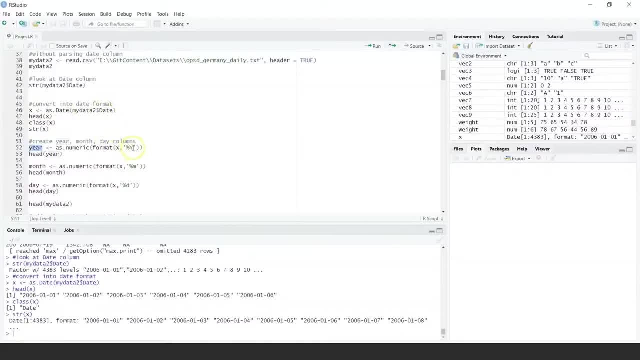 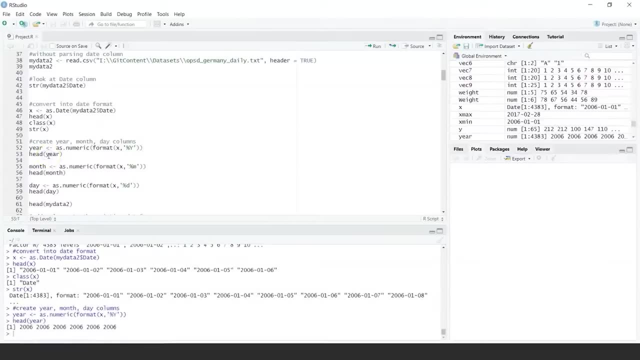 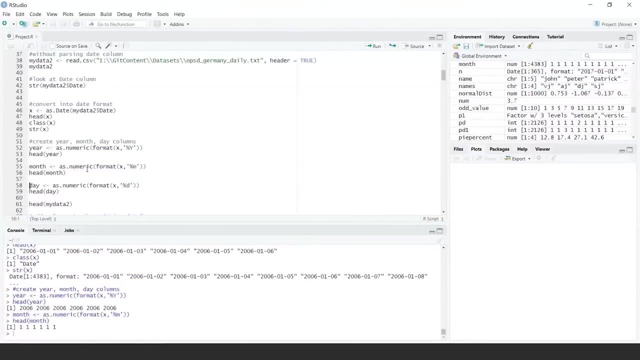 x, which is basically of date type, and then I am saying percentage y. so that will get me the year component out of this. let's look at the values. that shows me year component now. similarly, we can get the month out of this and then basically look at the month values. 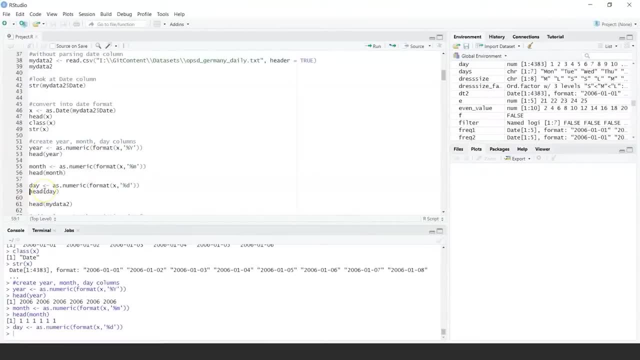 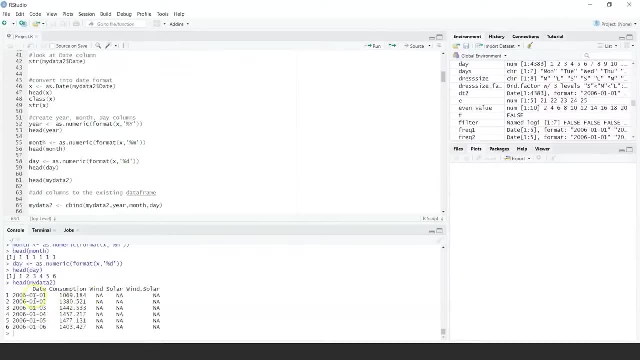 we can get the day out of it and we can get the day component. now, if I look at my data 2, which we had created earlier, this basically had date consumption, wind solar, wind solar. so what I can do is I can add these extracted columns such as year, month. 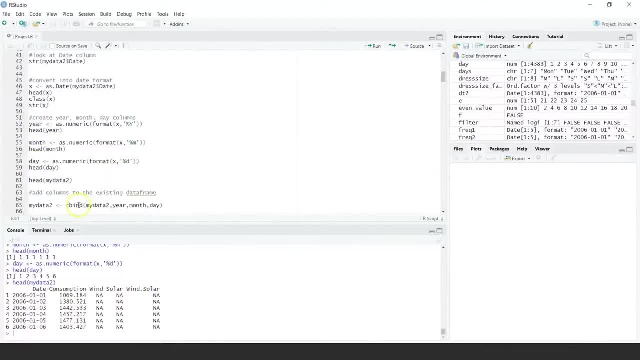 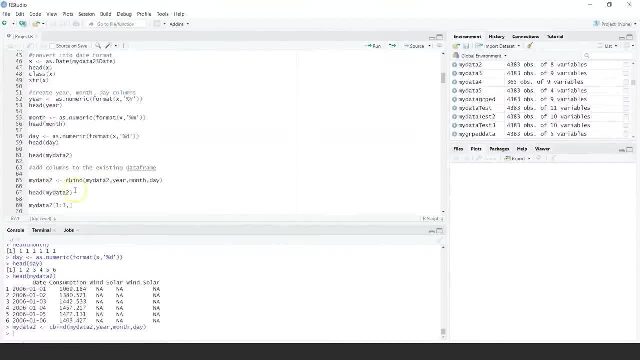 day to my data frame using a c bind, that is, column bind, and I will assign it to my data 2 again. so let's do this. and now, if you look at head, it shows me date, so that should be date format: consumption. now, this one might not. 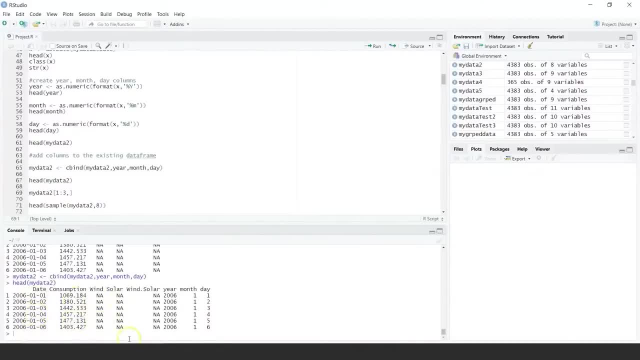 be date format, but we will see. you have consumption, wind, solar, and we have extracted the year, month and day which can help us for group by we can do some aggregations, we can do a plotting and we can do various things by these additional columns. now let's look at first 3 rows here. 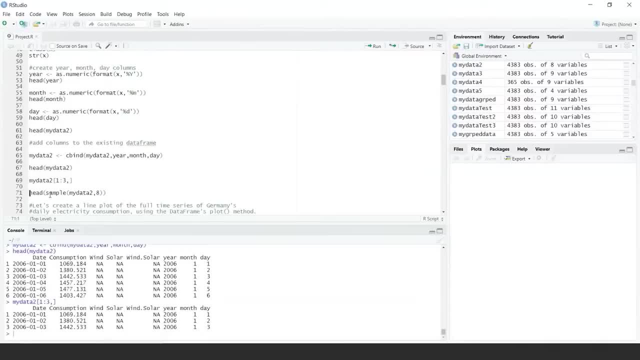 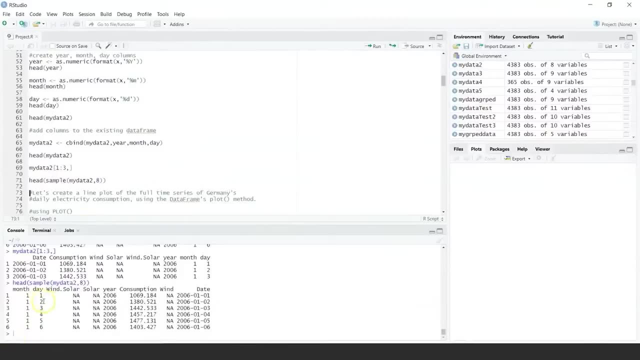 so I will say 1 is to 3, for my data 2, and that shows me some data. here you can always do a head and look at the sample of data. so that basically shows me month day, your columns and then you have your date now. 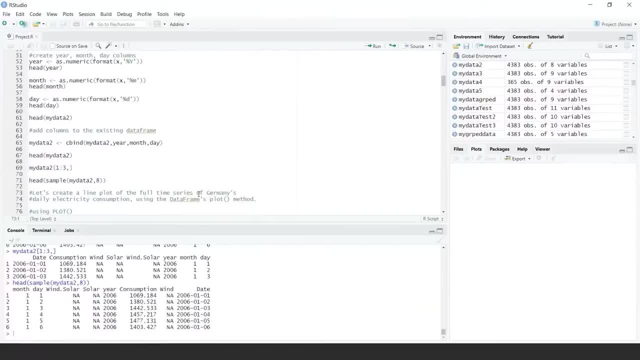 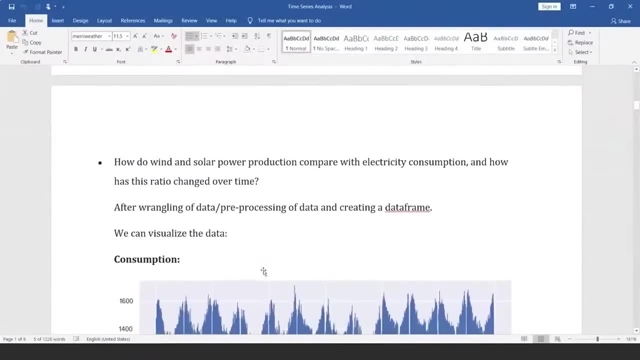 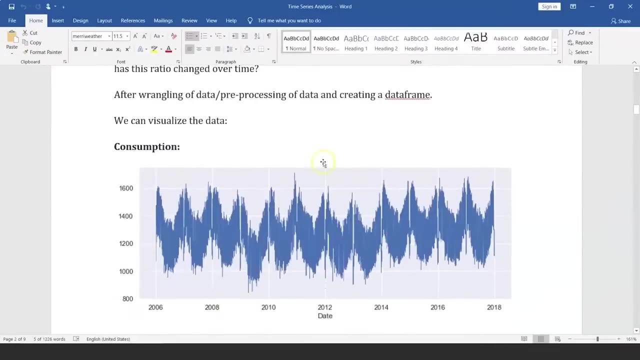 what we can do is we would want to visualize this data. we would want to basically understand the consumption. now, as I said, if we want to visualize the data, say, for example, I want this, which is consumption of data over years, and this one is in terms of: 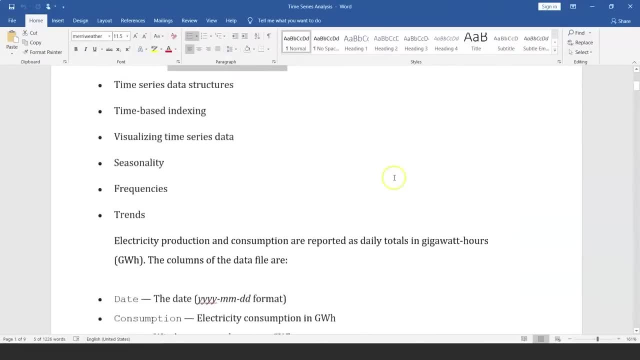 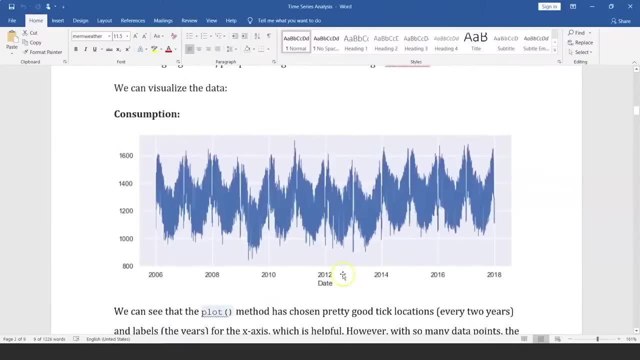 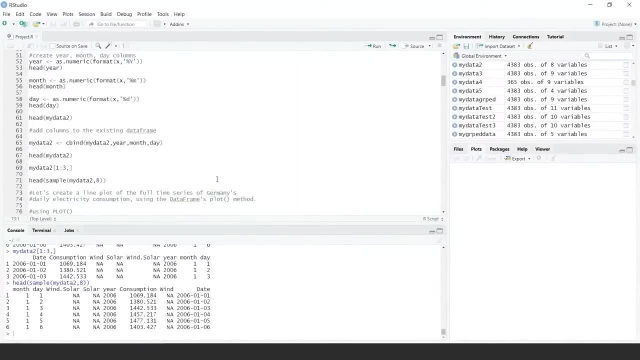 gigawatts per hour, as we were mentioning here gigawatt hours. so if I would want to create this visual to basically understand the pattern of the data, how do we do it? so we can you create a line plot of full time series of Germany's 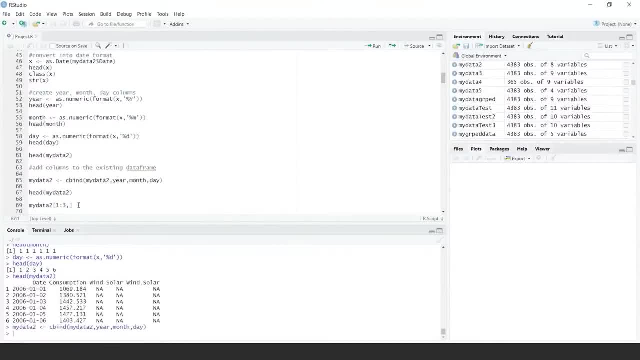 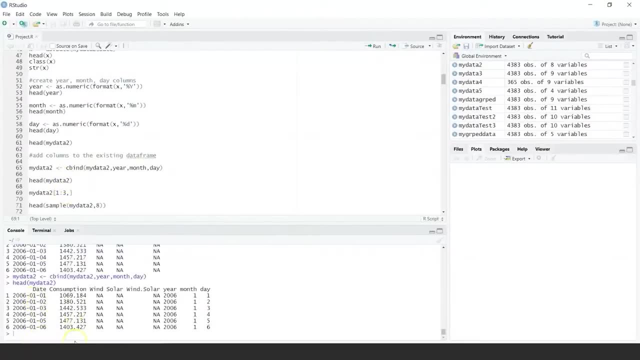 and I will assign it to my data 2 again. so let's do this. and now, if you look at head, it shows me date, so that should be date format. consumption: now, this one might not be date format, but we will see. you have consumption, wind, solar. 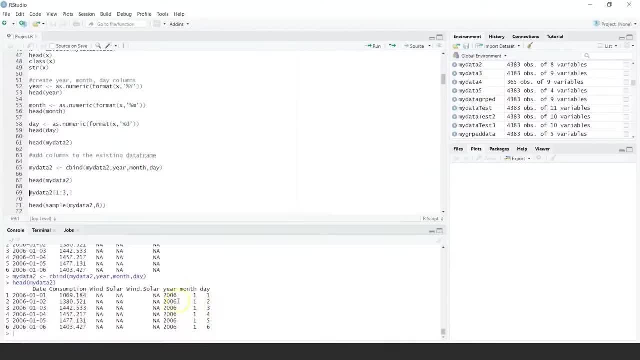 and we have extracted the year, month and day which can help us for group by we can do some aggregations, we can do a plotting and we can do various things by these additional columns. now let's look at first 3 rows here. so I will say 1 is to 3 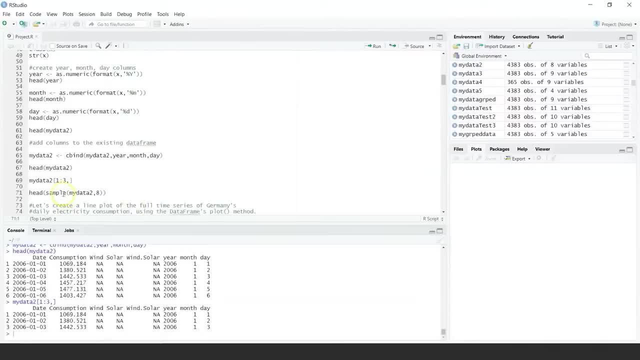 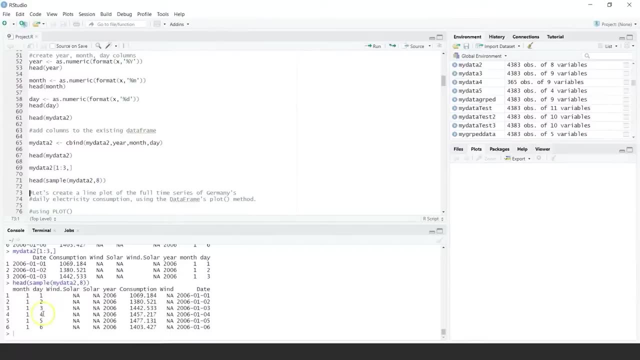 for my data 2 and that shows me some data. here you can always do a head and look at the sample of data, so that basically shows me month, day, your columns and then you have your date. now what we can do is: we would want to visualize this data. 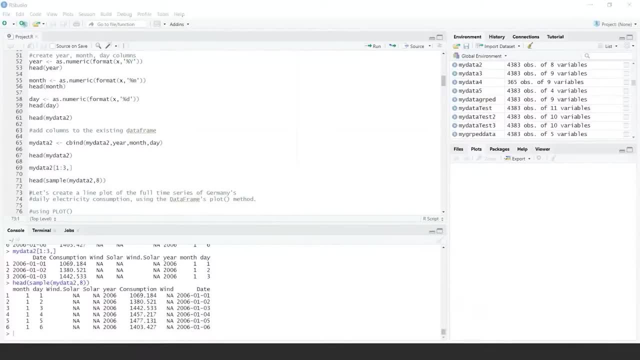 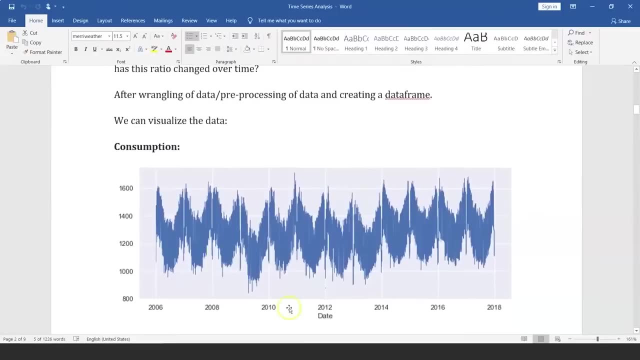 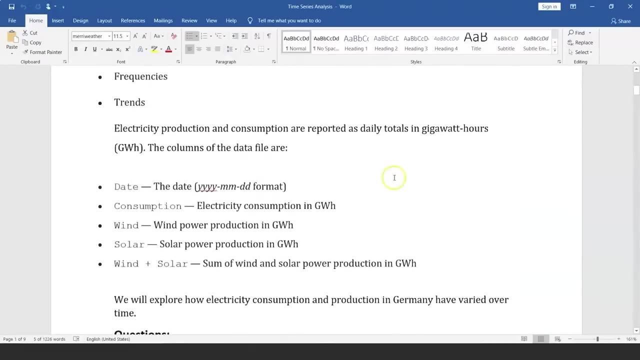 we would want to basically understand the consumption. now, as I said, if we want to visualize the data, say, for example, I want this, which is consumption of data over years, and this one is in terms of gigawatts per hour, as we were mentioning here. gigawatt hours: 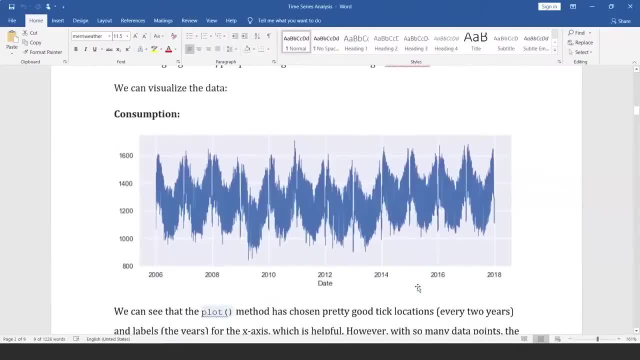 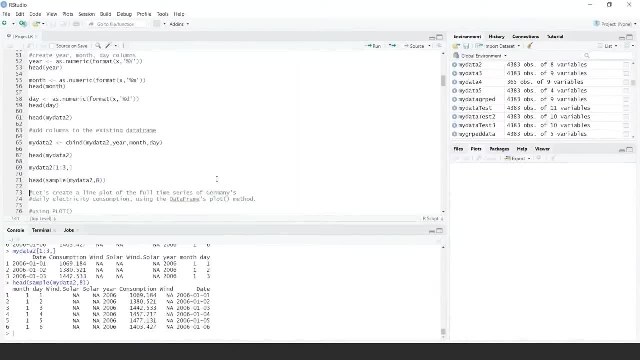 so if I would want to create this visual to basically understand the pattern of the data, how do we do it? so we can you create a line plot of full time series of Germany's electricity consumption using the plot method? now, how do we do that? so here, 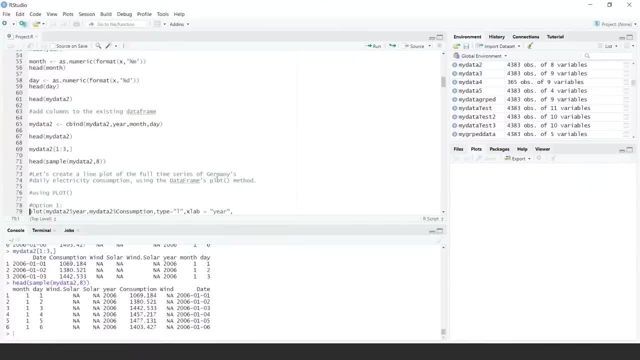 one of the option is I can straight away use the plot method. I can then say what would be in my x axis, what would be on my y axis, what would be the type of graph I would want to plot, what is my name on x axis, y axis and this. 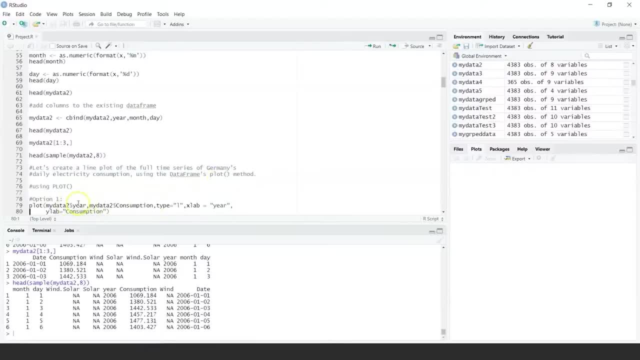 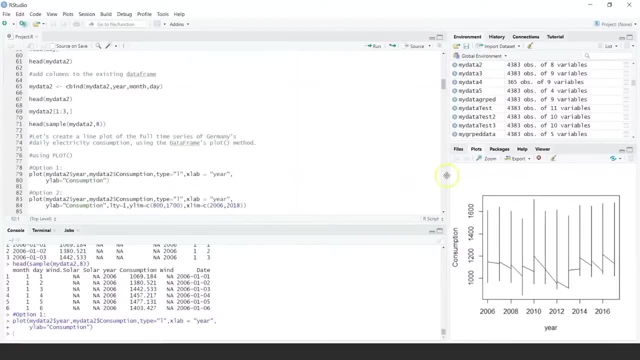 is the simplest way. so I am saying my data 2, I am extracting the year column and here I am taking the consumption. so let's create a plot. and here, if you see, we are looking at a plot, we do see some tick times and we see: 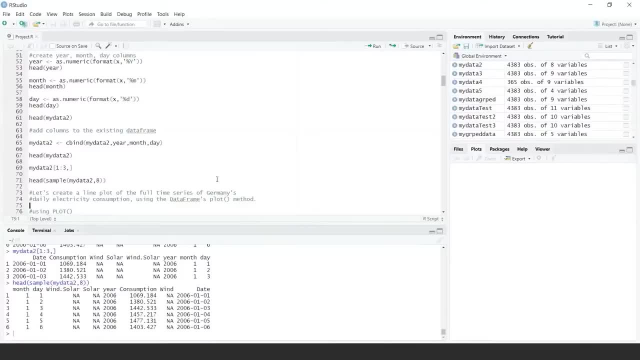 electricity consumption using the plot method. now, how do we do that? so here one of the option is: I can straight away use the plot method. I can then say what would be in my x-axis, what would be on my y-axis, what would be the type of 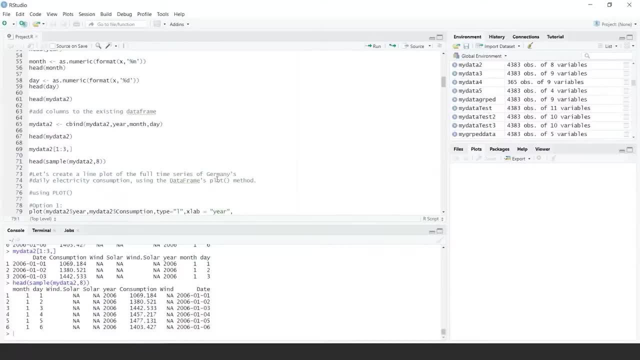 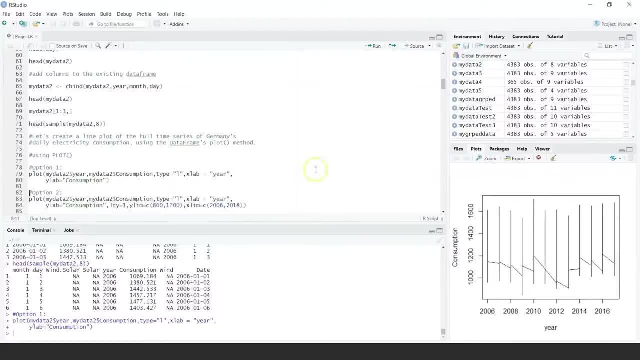 graph. I would want to plot what is my name on x-axis, y-axis, and this is the simplest way. so I am saying my data to, I am extracting the year column and here I am taking the consumption. so let's create a plot and here, if you see, we are looking. 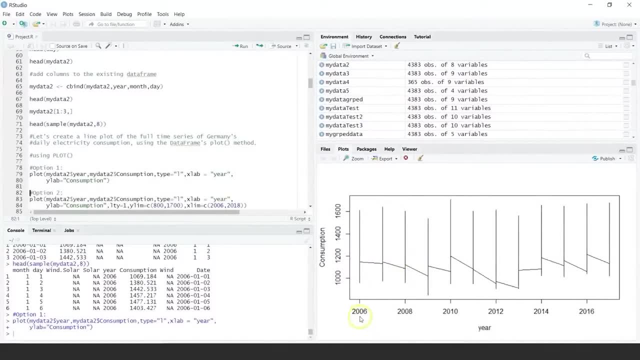 at a plot. we do see some tick times and we see that the data has been divided with every two years, so from 2006 onwards to 2016, but then really, this data does not give me, you know, a very useful way of looking at the data. 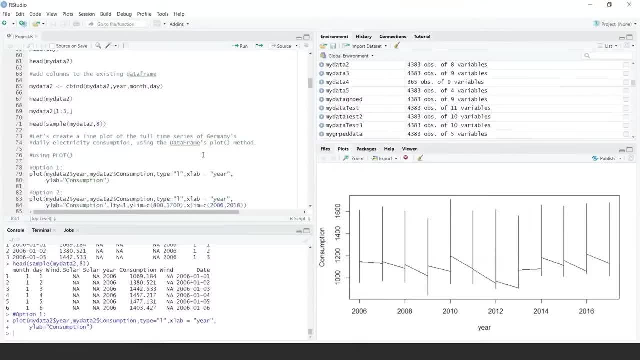 understanding it might be. what I can do is I can use the same way, but I can give, apart from x-axis and y-axis, I can say the limits, that is, x limit is 2006 to 2018 and y limit is from 800 to 1700. 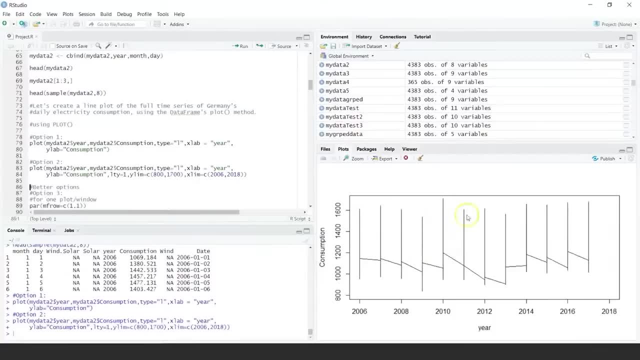 so we can do this and let's look at this again. this is a plot, but it really does not help me in visualizing and understanding the data. so what are the better options? I can go for multiple plots in a window. as of now, we are just sticking to one plot in window. 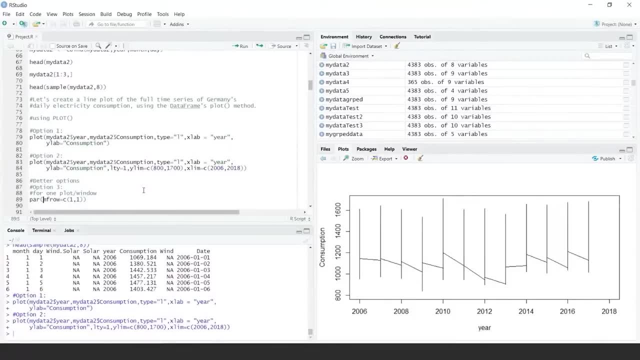 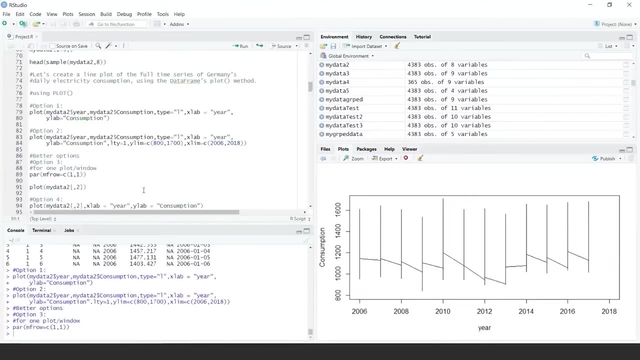 so if you would want to have multiple plots, you can always change the value here and make it 2 or 3. that will say how many rows and how many columns. as of now, we will just keep it as it is: par mf row. now, if I would want to plot, I can. 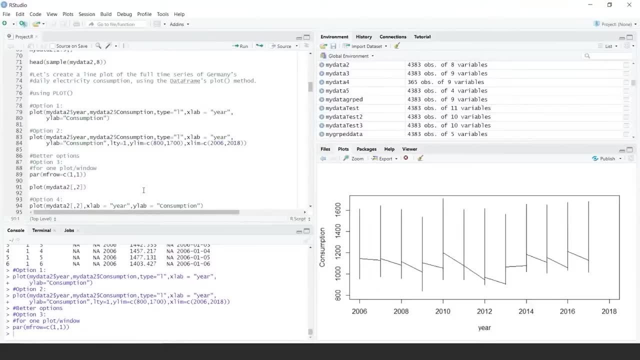 straight away give the column name. so I am interested in getting the consumption. now I can just do a plot. I will say my data 2 and I will choose the second column, which is consumption, which we saw here from our data. so consumption was the second column, so I can just 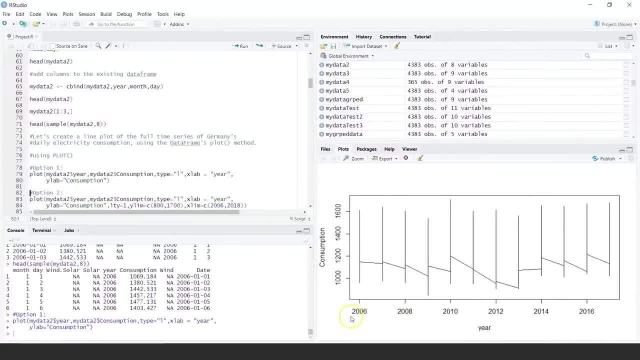 that the data has been divided with every 2 years, so from 2006 onwards to 2016, but then really this data does not give me a very useful way of looking at the data or understanding it might be. what I can do is I can. 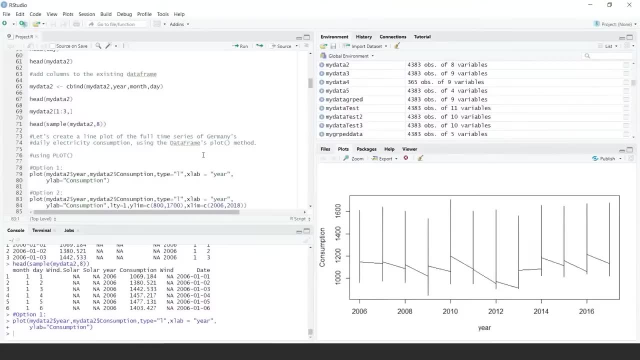 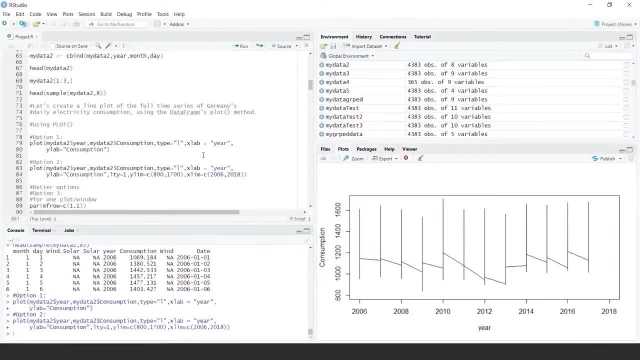 use the same way, but I can give, apart from x axis and y axis, I can say the limits, that is, x limit is 2006 to 2018 and y limit is from 800 to 1700. so we can do this and let's look at this again. this is: 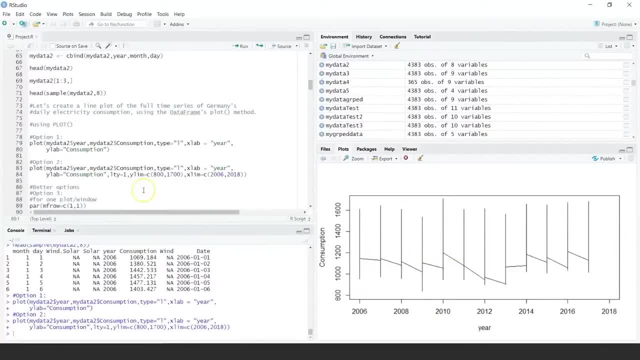 a plot, but it really does not help me in visualizing and understanding the data. so what are the better options? I can go for multiple plots in a window. as of now, we are just sticking to one plot in window. so if you would want to have multiple plots, you can. 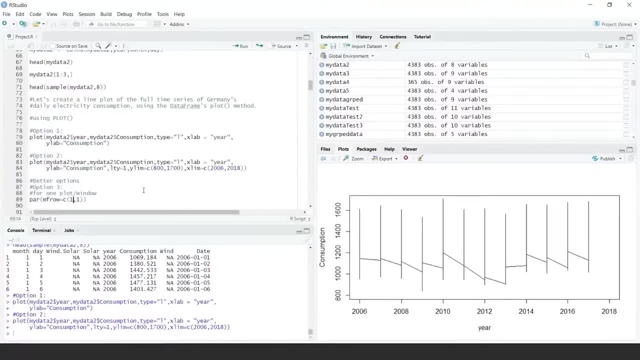 always change the value here and make it 2 or 3. that will say how many rows and how many columns. so as of now we will just keep it as it is. par mf row. now if I would want to plot, I can straight away give the column name. 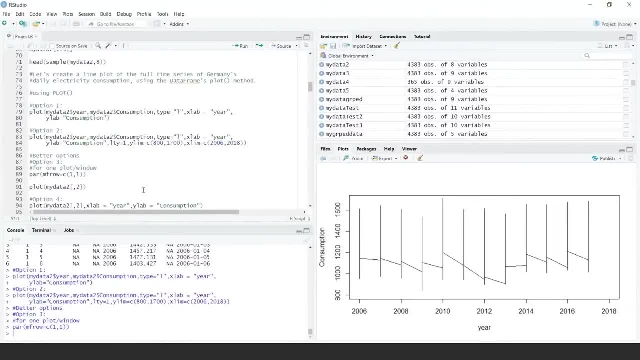 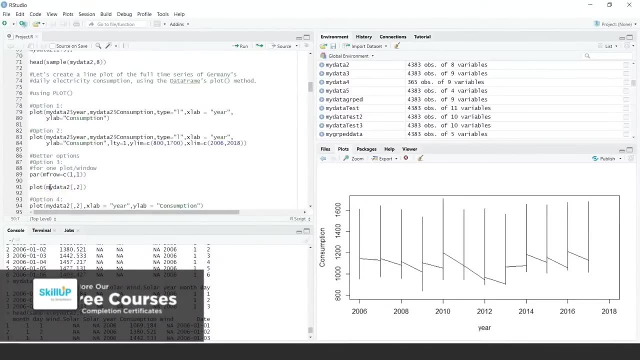 so I am interested in getting the consumption. now I can just do a plot. I will say my data 2 and I will choose the second column, which is consumption, which we saw here from our data. so consumption was the second column, so I can just do a plot in a straight away. 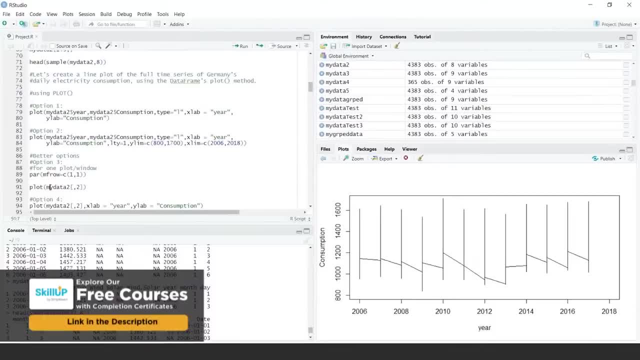 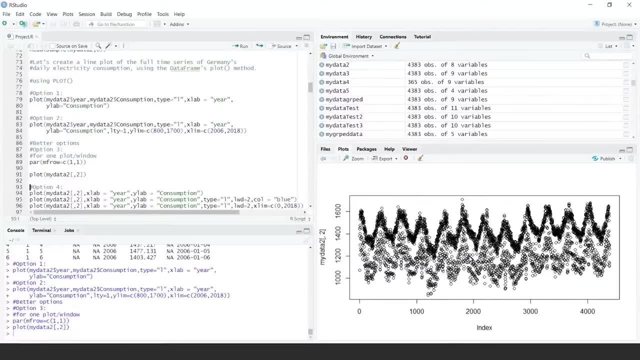 way, without mentioning your x axis, y axis, limits and so on. and if you look at this, this one is giving me a pattern. now, here I am looking at x axis, y axis, which is not really named- we do not have a name to this graph- and we are looking at the data it does. 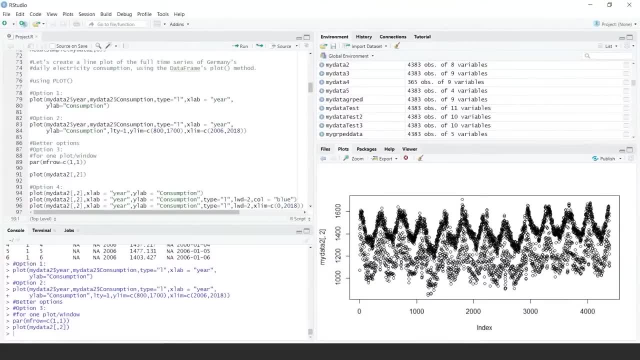 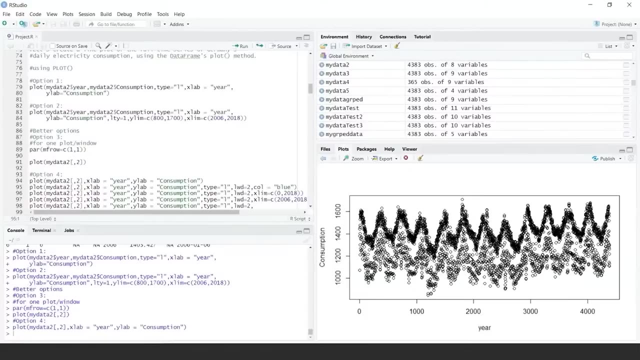 show me some kind of pattern, but might be we can make it more meaningful. so I can do it this way where I say my data, second column, lets give axis as year. x axis, y axis is consumption. now that has changed the x axis and y axis. now I can also give 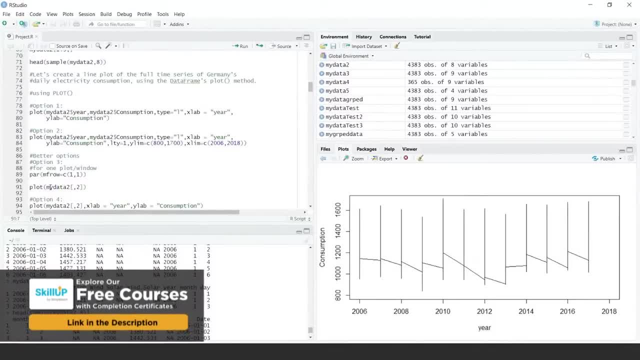 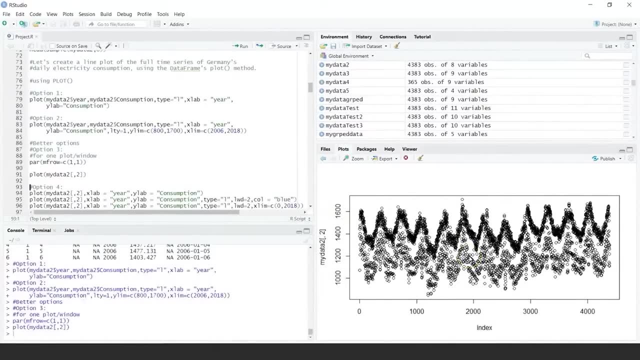 do a plot in a straight away way, without mentioning your x-axis, y-axis, limits and so on, and if you look at this, this one is giving me a pattern. now, here I am looking at x-axis, y-axis, which is not really named- we do not have a name to this graph. 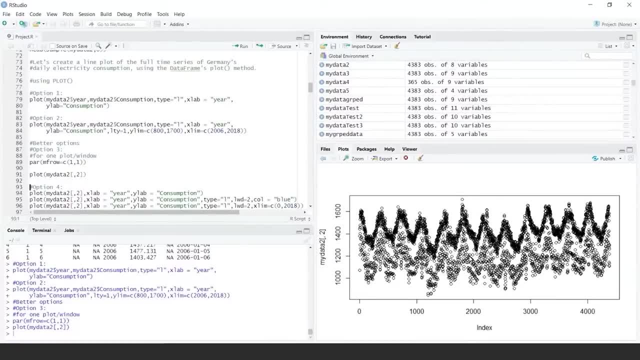 and we are looking at the data. it does show me some kind of pattern, but might be we can make it more meaningful. so I can do it this way, where I say my data. second column: let's give axis, as here: x-axis, y-axis is consumption. now that has 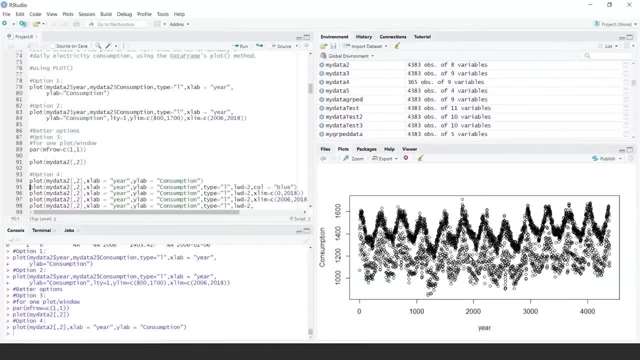 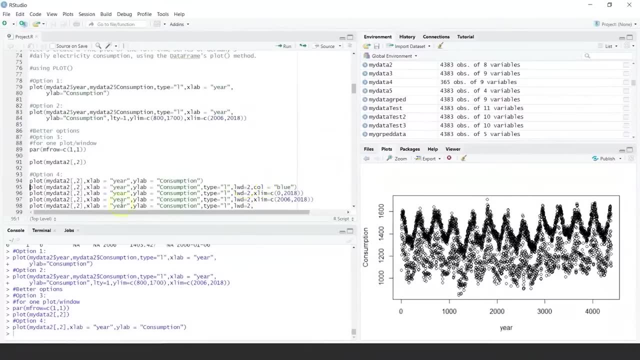 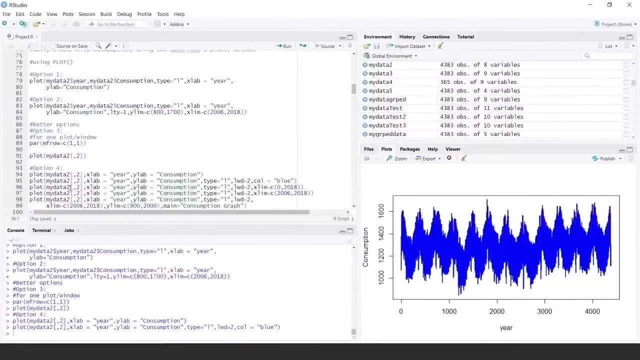 changed the x-axis and y-axis. now I can also give some more details. I can say: type should be line. I have the line width. I am saying color is blue and let's do this so this looks more meaningful. might be: shows a wavering pattern of consumption over years. 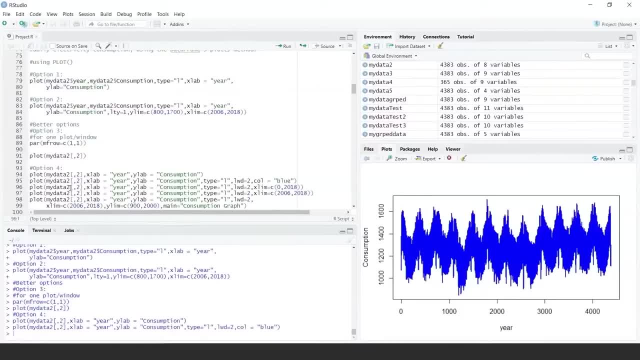 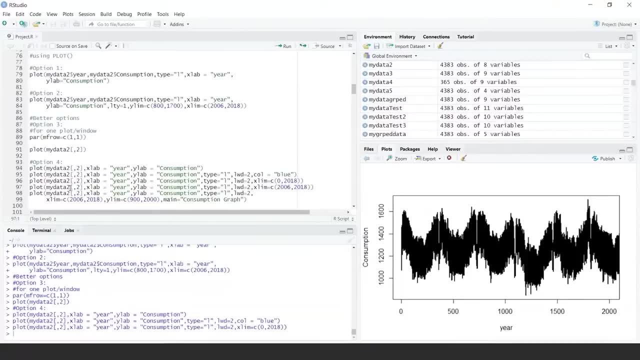 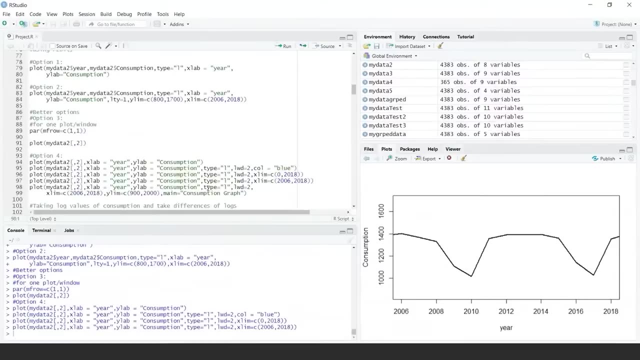 I can also give a limit of x that is 0 to 2018 and that basically shows me the range. now we can change that and we can be more specific and saying x limit should be 2006 to 2018. and let's look at this. 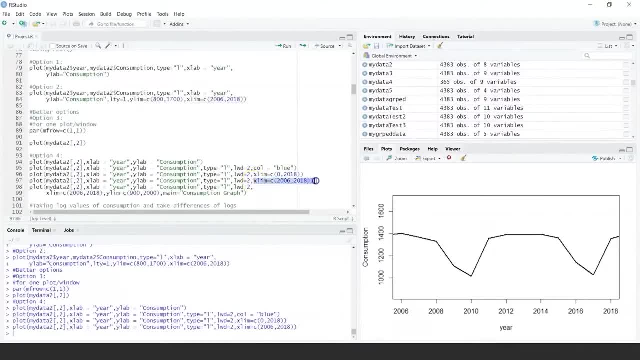 now this one, once you have given a proper limit. it shows the line graph and it shows what was the consumption in 2006 and over a period till 2018. I can then use any. of these. options are fine, but it depends on what and whom. 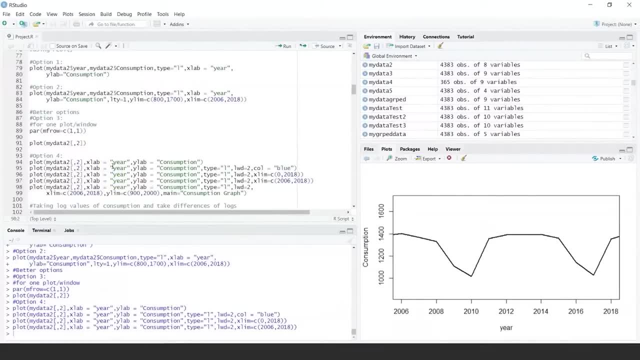 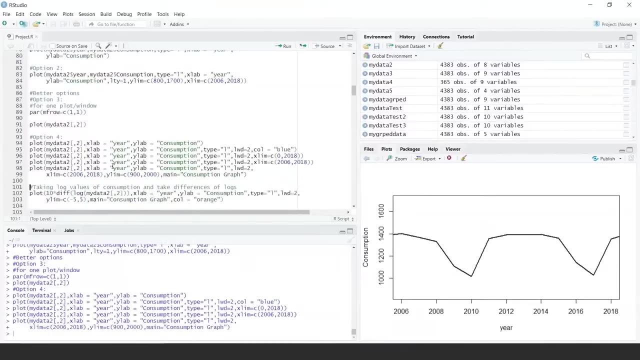 you are presenting the data or what kind of analysis you are doing. so I can do a plot. I can choose column second, x lab, which is x-axis, y-axis, type, is line width, giving x limit, y limit. and then I am giving a title to this, which is consumption graph. 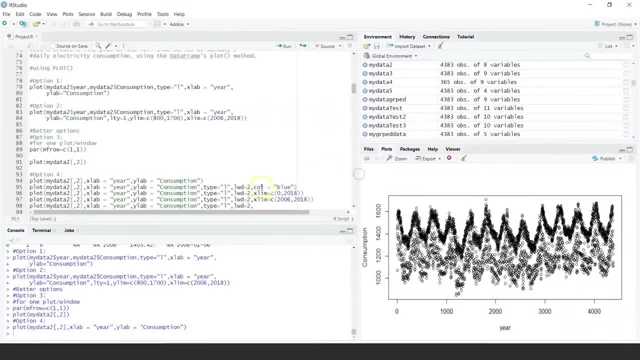 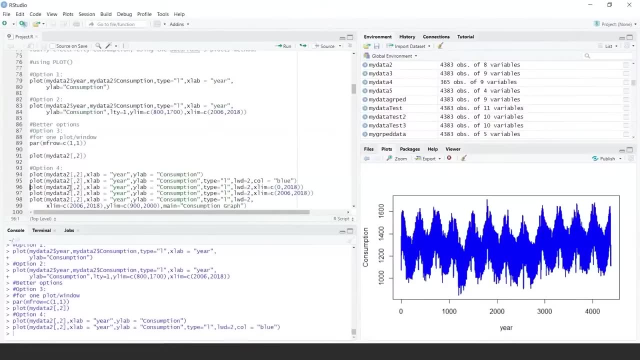 some more details. I can say type should be line. I have the line width. I am saying color is blue and lets do this so this looks more meaningful. might be shows a wavering pattern of consumption over years. I can also give a limit of x that is 0 to. 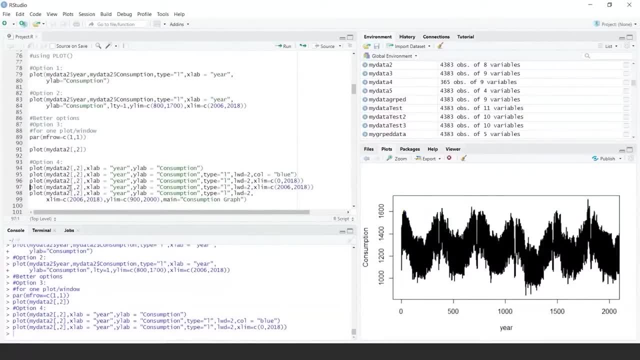 2018 and that basically shows me the range. now we can change that and we can be more specific and saying x limit should be 2006 to 2018. and lets look at this now, this one: once you have given a proper limit, it shows: 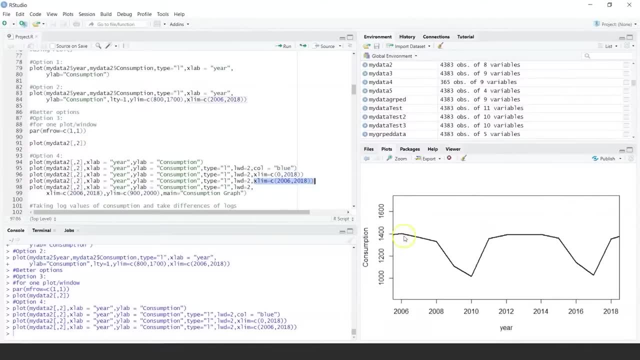 the line graph and it shows what was the consumption in 2006 and over a period till 2018. I can then use. any of these options are fine, but it depends on what and whom you are presenting the data or what kind of analysis you are doing. 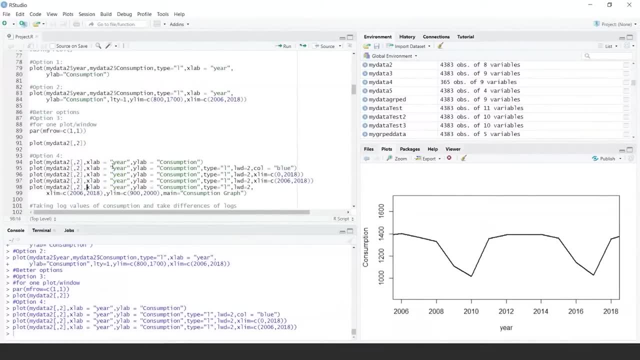 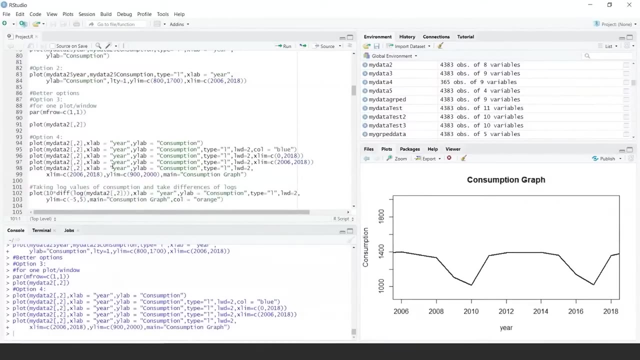 so I can do a plot. I can choose column second, x lab, which is x axis, y axis, type is line width, giving x limit, y limit, and then I am giving it title to this, which is consumption graph, and then basically you are looking at the line graph. 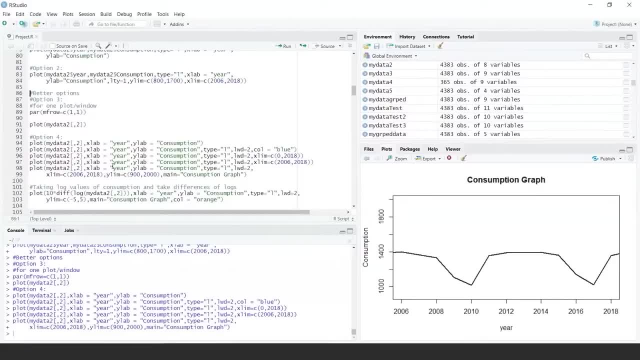 now those are the options which you can do. either you could be very specific, or you could just give your column which you want to plot, or obviously, make it more meaningful by giving all the details. now, what we can do is, if we would want to look at 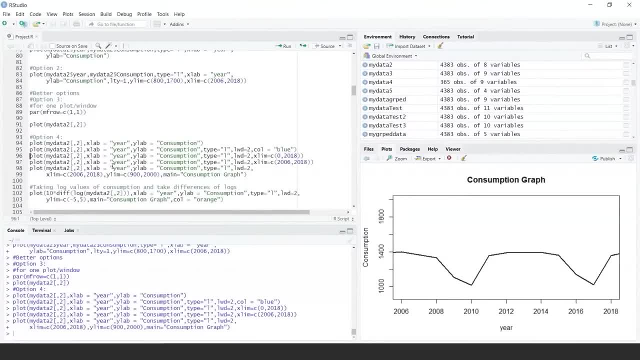 this data and understand it better, rather than just looking at a simple line. I can take the log values. so here I am saying log of my data to second column, so I am taking log values of consumption and I am taking the difference of logs, so I can. 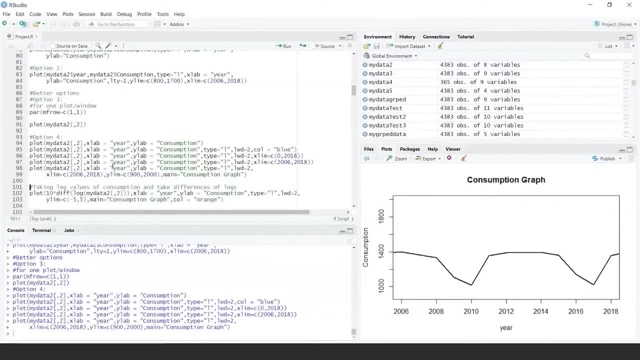 and then, basically, you are looking at the line graph. now those are the options which you can do. either you could be very specific, or you could just give your column which you want to plot, or obviously make it more meaningful by giving all the details. now, what we can do is 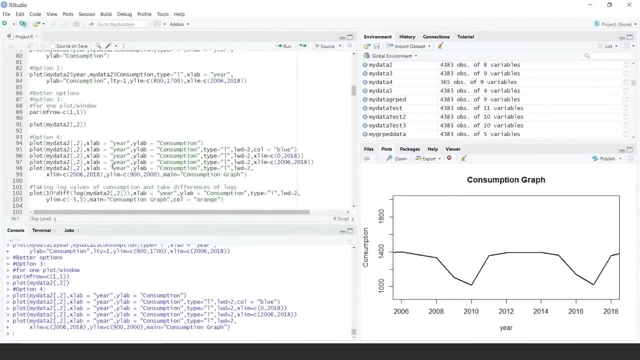 if we would want to look at this data and understand it better rather than just looking at a simple line, I can take the log values. so here I am saying log of my data- to second column. so I am taking log values of consumption and I am taking the difference. 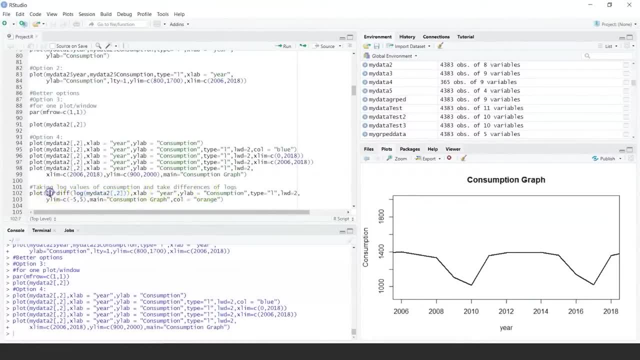 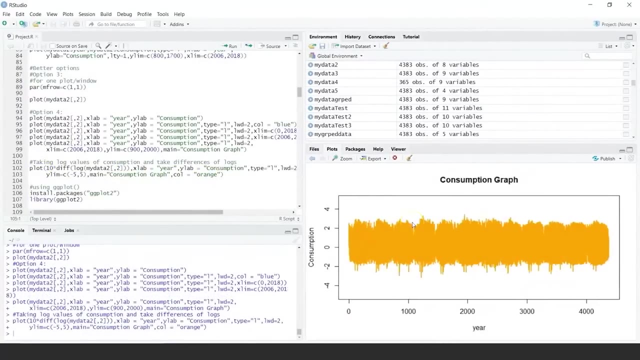 of logs, so I can say difference and then you can basically increase or decrease this by multiplying it by some number, so rest remains the same. I am changing the color and let's look at this plot and you see, this basically is giving me a better pattern, which 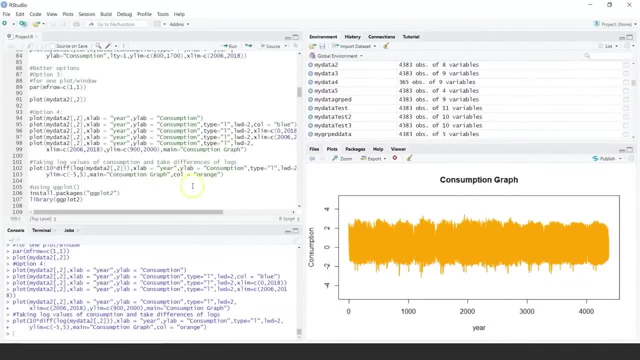 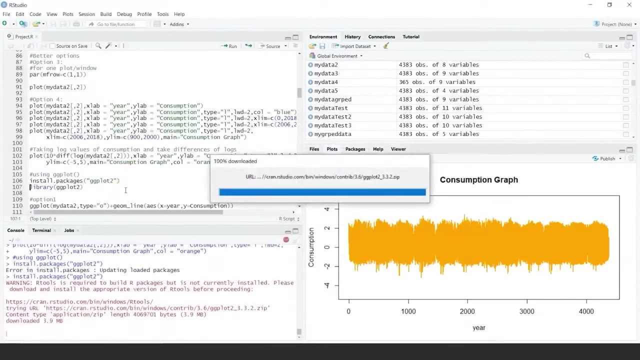 makes meaning. here we see the log values. so this is: you are using a simple plot function in R. you can also use ggplot. now for that, we can install the ggplot package. it's already there in my machine, so I will say no, I will access this by using the. 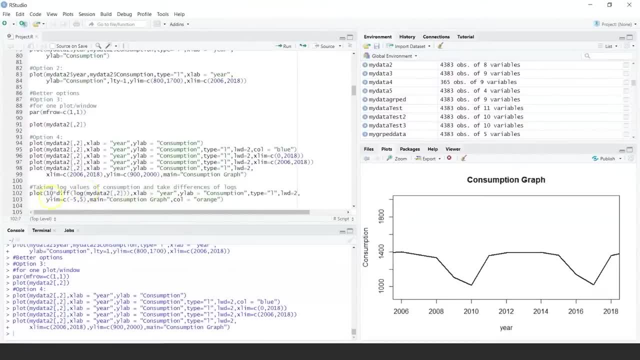 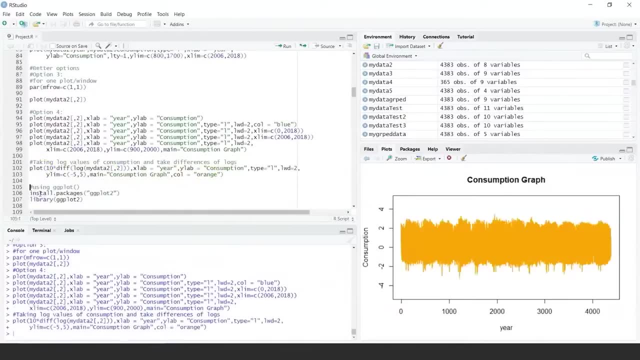 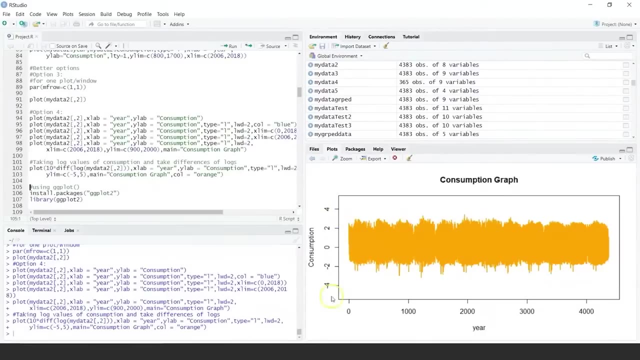 say difference, and then you can basically increase or decrease this by multiplying it by some number. so rest remains the same. I am changing the colour and let's look at this plot and you see this basically is giving me a better pattern, which makes meaning. here we see the 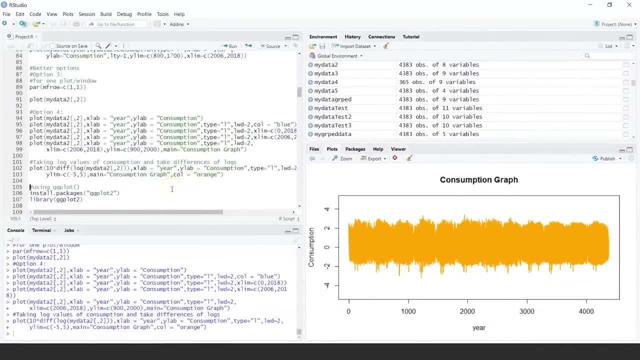 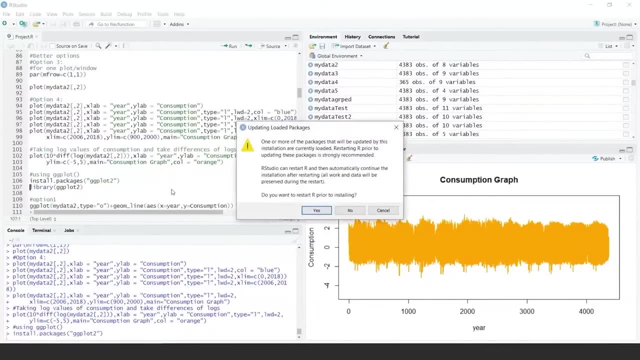 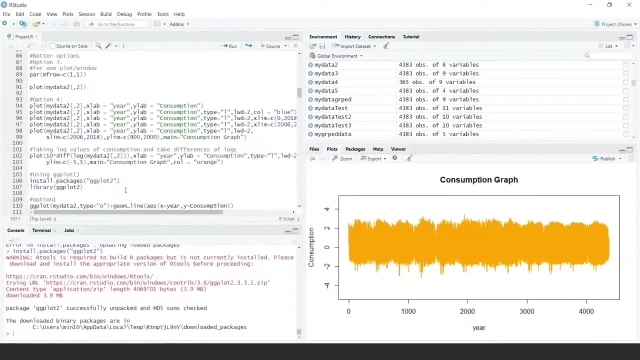 log values. so this is: you are using a simple plot function in R. you can also use ggplot. now for that, we can install the ggplot package. it's already there in my machine, so I will say no, I will access this by using the library ggplot. 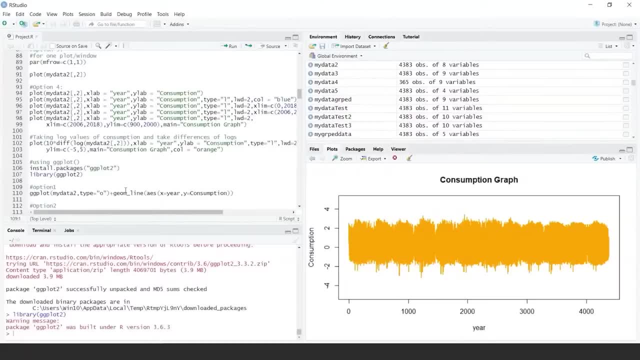 to, and now I can use ggplot to plot. so the way you specify here you can say my data to. that's the data frame. I am saying type as o and when I am saying line, I am basically going to use x axis, which is year, y is consumption. 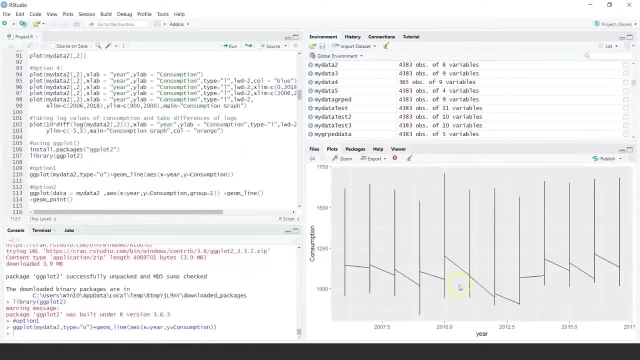 and let's look at this plot. so again we are back to the one which we were doing earlier. really does not make any sense, gives us some data but then really does not give me enough information. I can in my aesthetics, I can say x is year, y is. 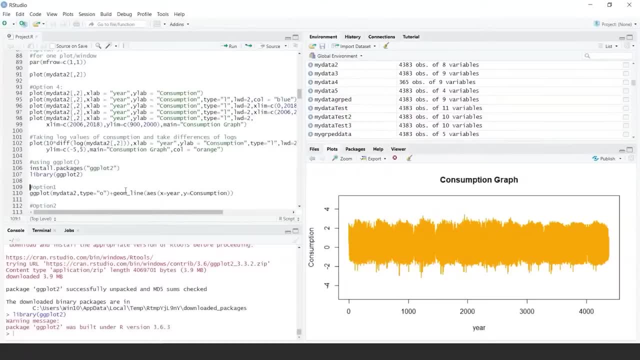 library ggplot2, and now I can use ggplot2plot. so the way you specify here, you can say mydata2, that's the data frame. I am saying type as o and when I am saying line, I am basically going to use x-axis, which is. 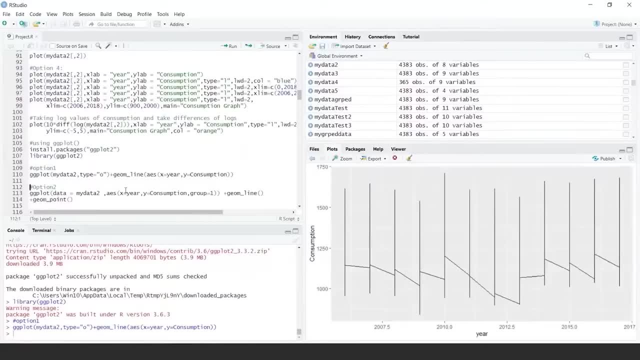 year y is consumption. and let's look at this plot. so again we are back to the one which we were doing earlier. really does not make any sense, gives us some data, but then really does not give me enough information. I can in my aesthetics, I can say: 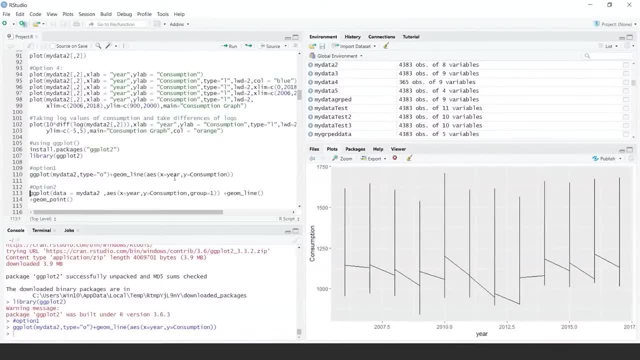 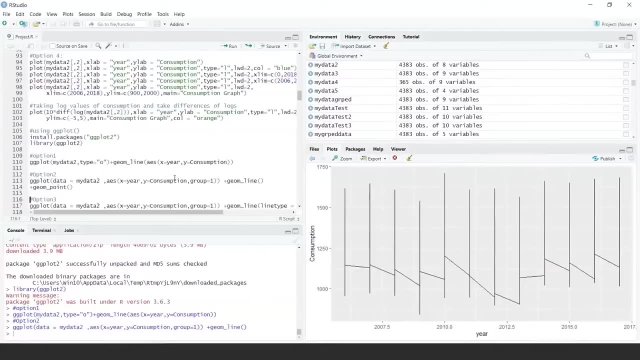 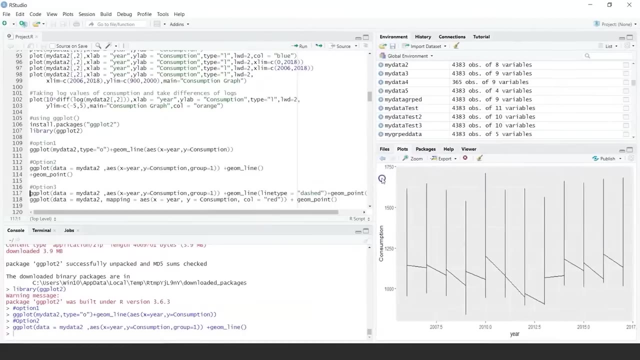 x is year, y is consumption. I can do a grouping and then I can give line and plot. so again, we have some information, but really does not help me right now. let's look at other example. so I am just doing the same thing here and I am looking at line. 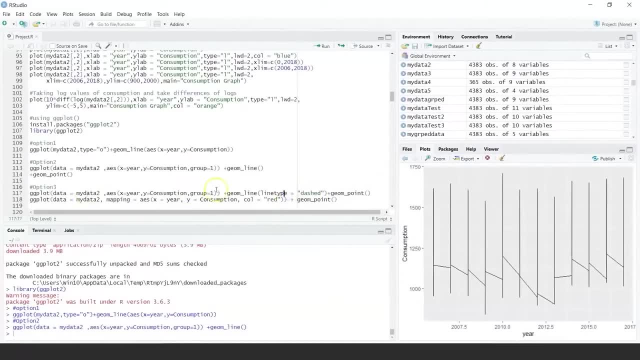 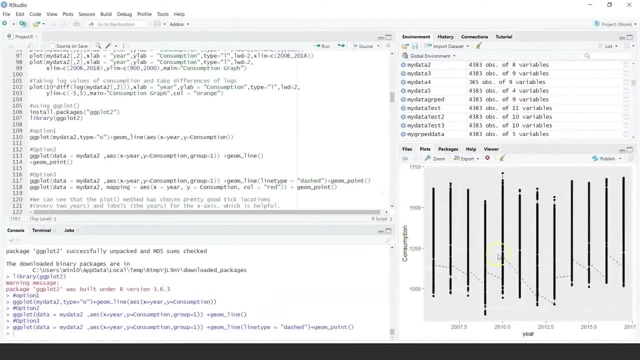 type being dashed. I am using the ggplot, other methods such as geomline and quantum point to give me more information and if I look at the plot, it does give me data. it tells me what are the different values. it gives me some kind of pattern. but 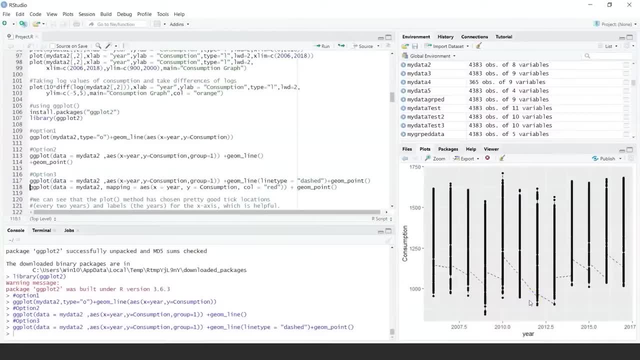 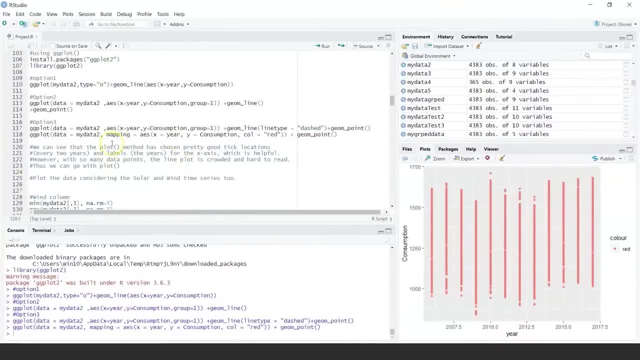 I would still prefer the way we were doing with plot. now we can change the color and obviously add details to it. so what we see is when you use the plot method, which I did earlier, it was choosing pretty good tick locations. that is every two years, and labels the years for. 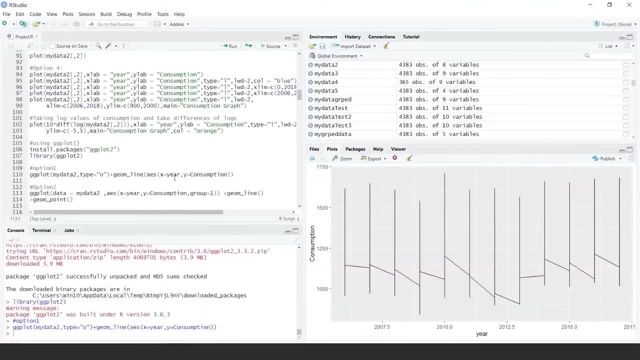 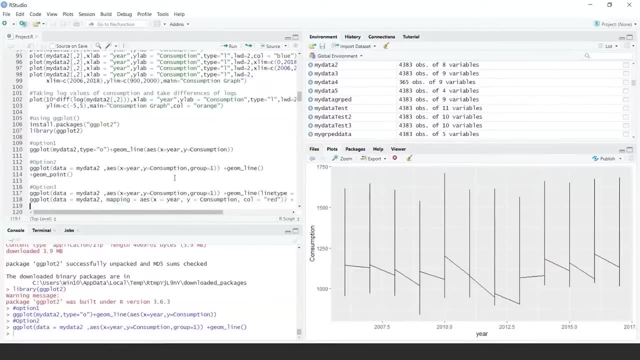 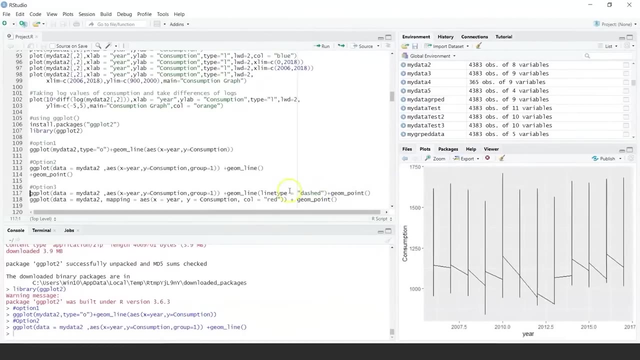 consumption. I can do a grouping and then I can give line and plot. so again, we have some information, but really does not help me right now. let's look at other example. so I am just doing the same thing here and I am looking at line type being dashed. 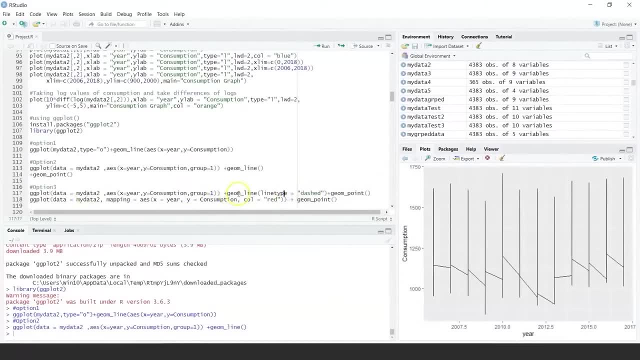 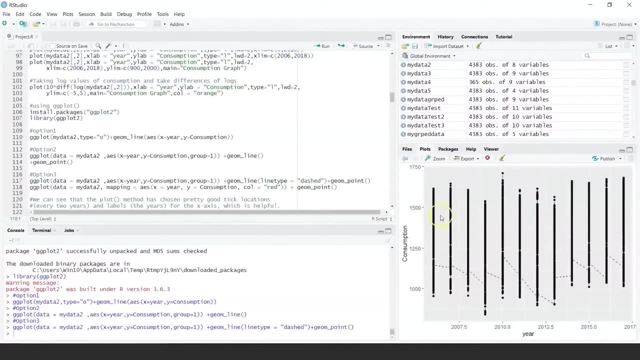 I am using the ggplot, other methods such as geomline and geompoint, to give me more information and if I look at the plot, it does give me data. it tells me what are the different values. it gives me some kind of pattern, but I would still prefer the way. 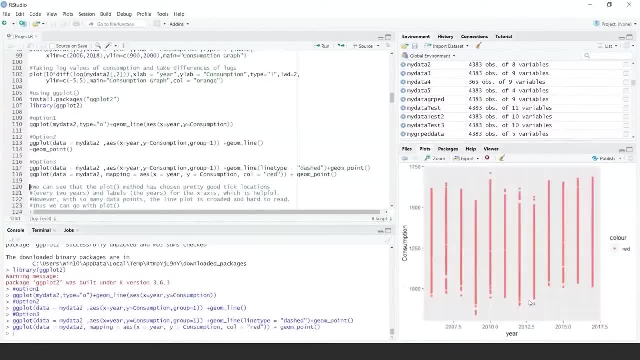 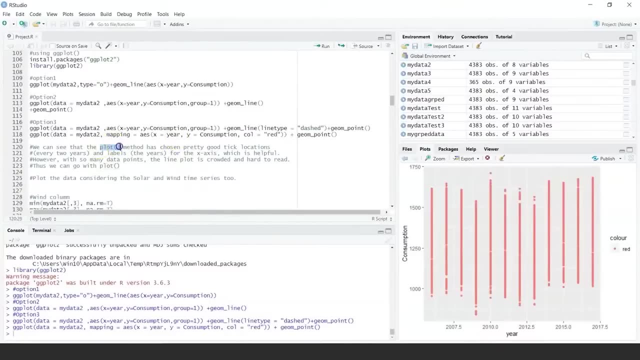 we were doing with plot. now we can change the color and obviously add detail to it. so what we see is, when you use the plot method, which I did earlier, it was choosing pretty good tick locations, that is every two years, and labels the years for the x axis, which was 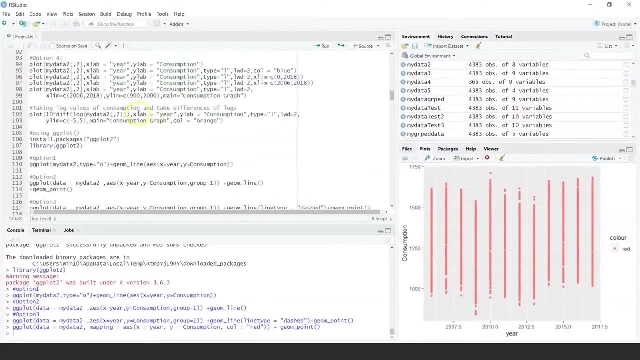 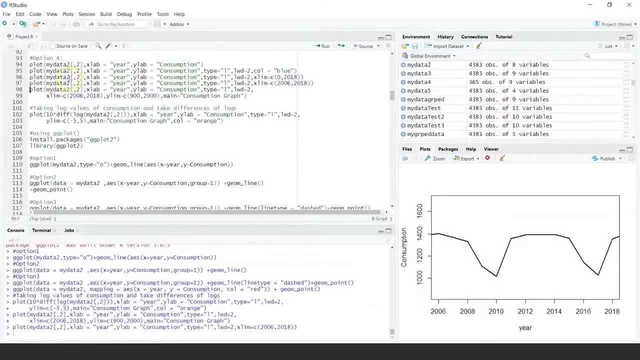 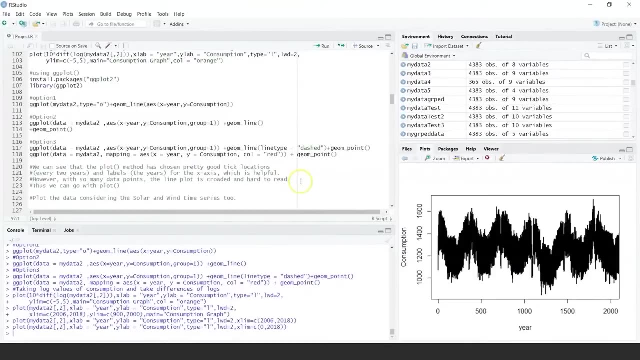 helpful, right, but with these data points which we were seeing here or say, for example, this one, or say this one, or say this one, we are looking at some data, but then that real is quite crowded and it is hard to read. you can look at the values, but then 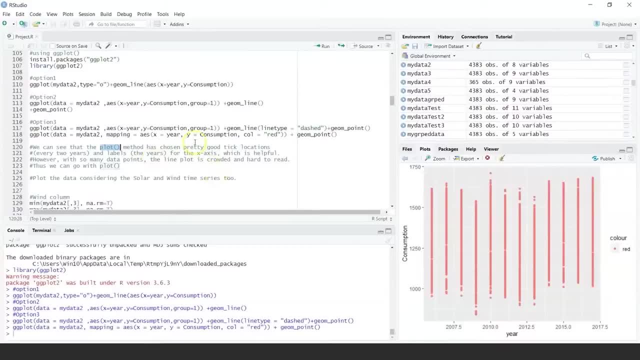 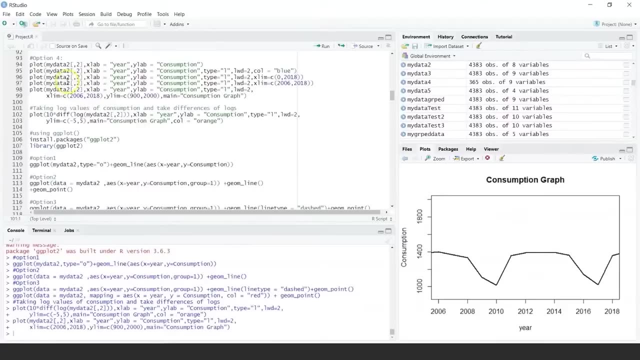 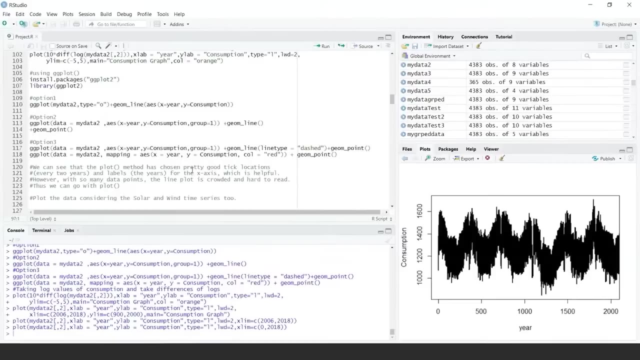 the x axis, which was helpful, right, but with these data points which we were seeing here or say, for example, this one, or say this one, or say this one, we are looking at some data, but then that really is quite crowded and it is hard to read. you can. 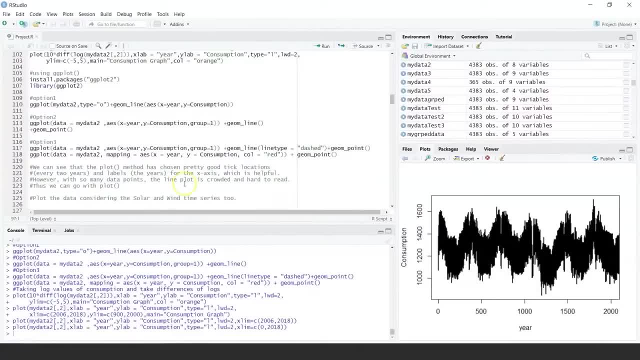 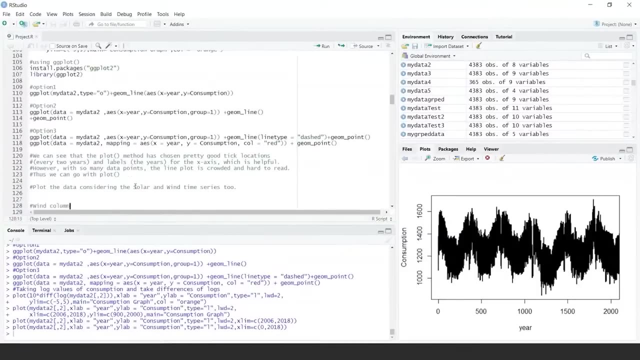 look at the values, but then it really does not give you enough information. so we can go for plot method, but then we will see how we can consider different data. now if I would want to plot the solar and wind time series, so let's see how do we do that. 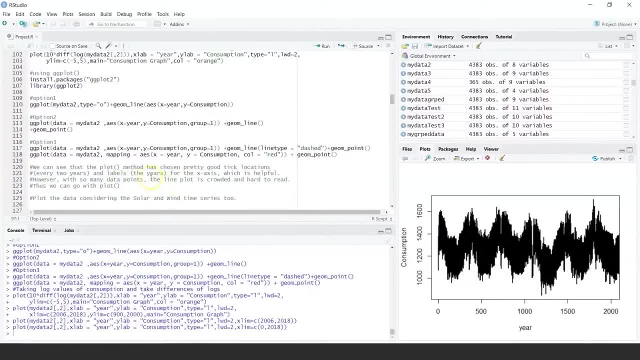 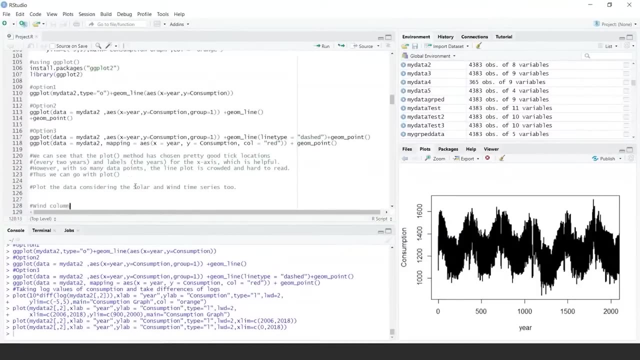 it really does not give you enough information. so we can go for plot method, but then we will see how we can consider different data. now if I would want to plot the solar and wind time series, so let's see how do we do that. so wind column. 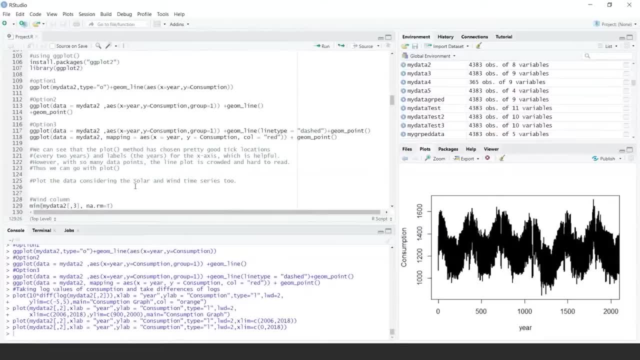 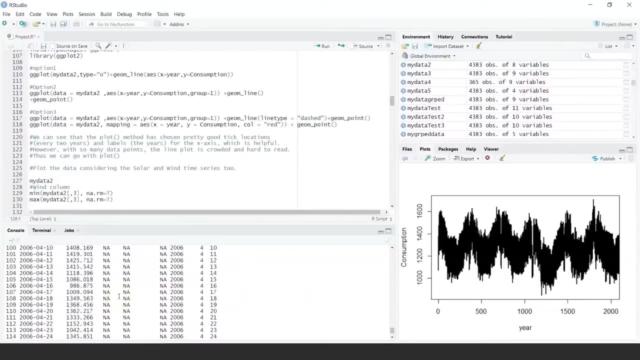 is what I am interested in. so first thing is it was always good to find out the minimum and the maximum values in every column. so I am saying minimum, I am saying let's put in here my data. two, and then let's look at the values. so we are looking at. 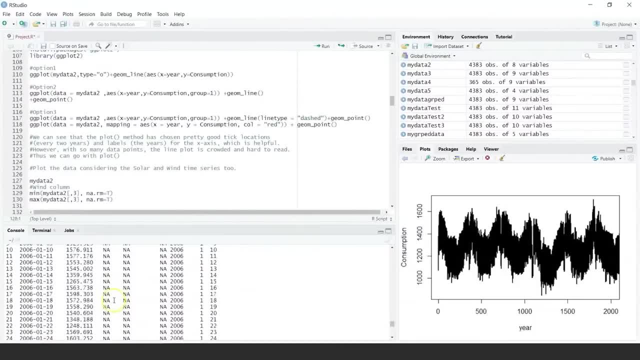 the columns we know: consumption is the second column, wind is the third column and you have solar is the fourth and this one is the fifth. so let's say, let's find out the minimum of each of these columns which we would want to plot. so let's. 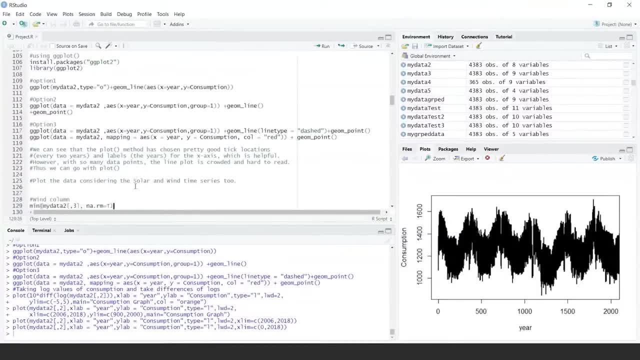 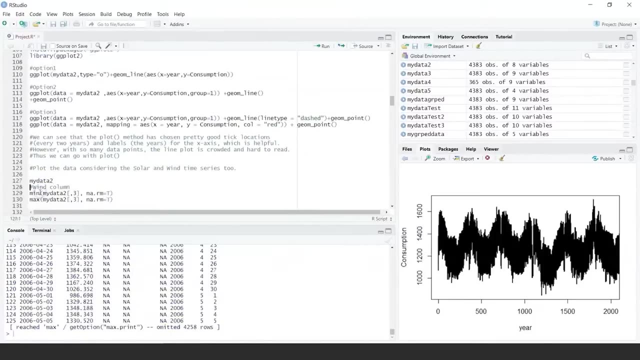 so wind column is what I am interested in. so first thing is it was always good to find out the minimum and the maximum values in every column. so I am saying minimum, I am saying let's put in here my data 2, and then let's look at 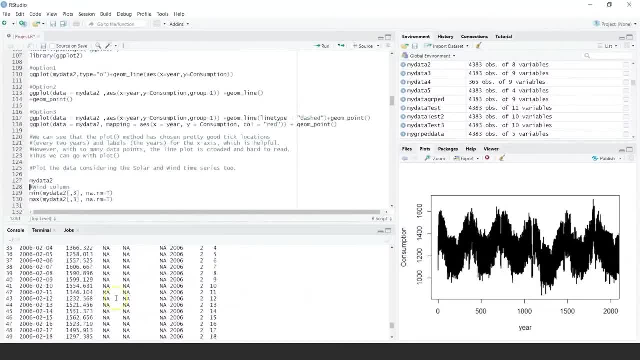 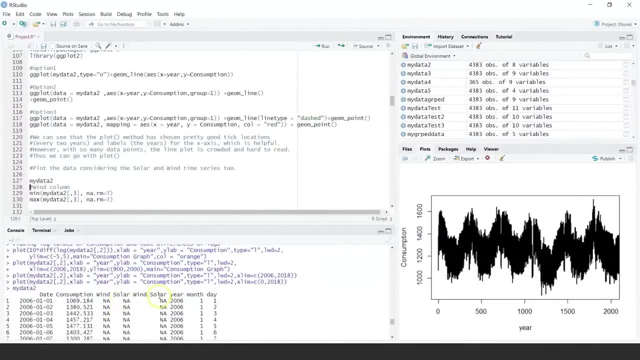 the values. so we are looking at the columns. we know consumption is the second column, wind is the third column and you have solar is the fourth and this one is the fifth. so let's say, let's find out the minimum of each of these columns which we would 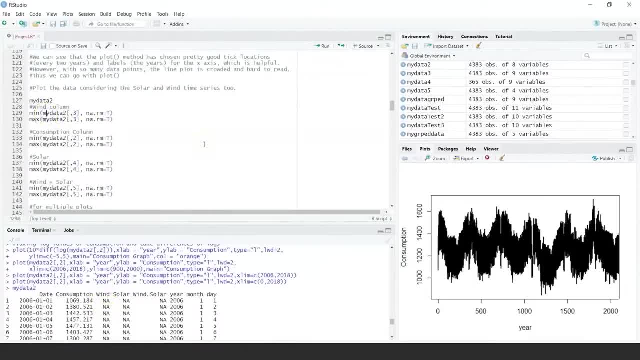 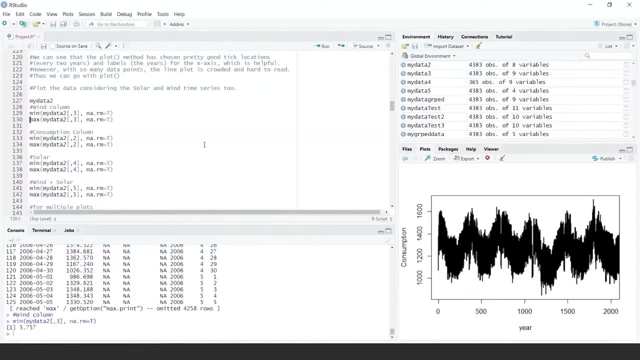 want to plot. so let's say: minimum of data, third column. and here I am also saying: remove the NA values, because we do not want to consider the NA values. so let's look at the minimum. that shows me 5.757. what is the maximum value? it is 826. 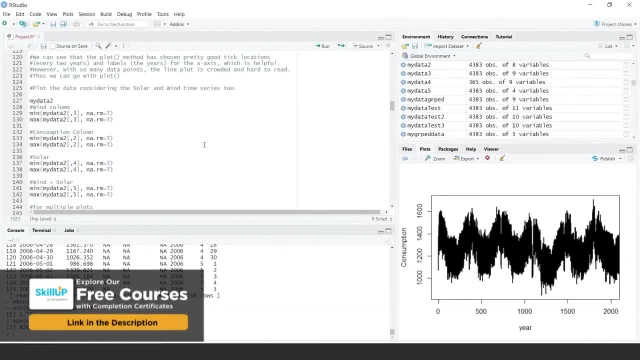 so that also helps me in giving a limit. if I want to plot wind on y axis, I can give a y limit from 5 to 850. consumption wise, let's find out the minimum from second column and maximum and similarly for solar find the minimum and maximum. 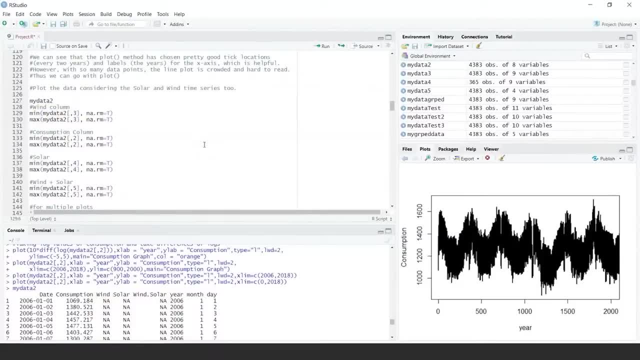 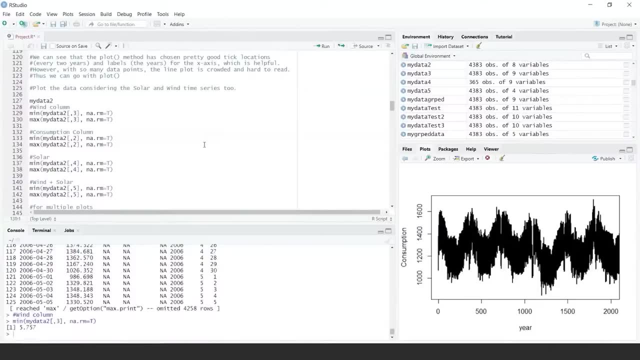 say minimum of data, third column, and here I am also saying: remove the NA values, because we do not want to consider the NA values. so let's look at the minimum. that shows me 5.757. what is the maximum value? it is 826. so that also helps me in giving a. 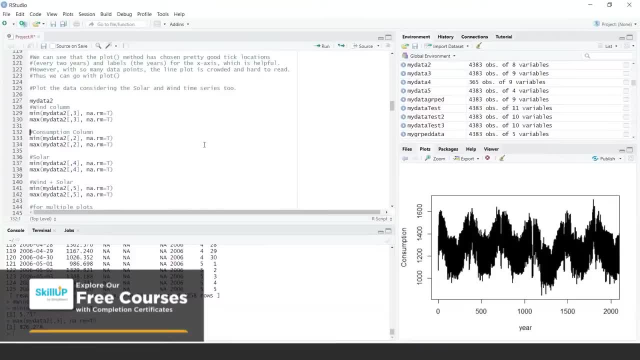 limit. if I want to plot wind on y axis, I can give a y limit from 5 to 850. consumption wise, let's find out the minimum from second column and maximum and similarly for solar find the minimum and maximum and wind plus solar minimum and maximum. so 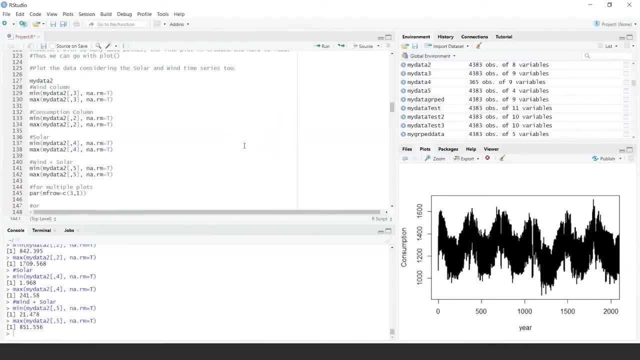 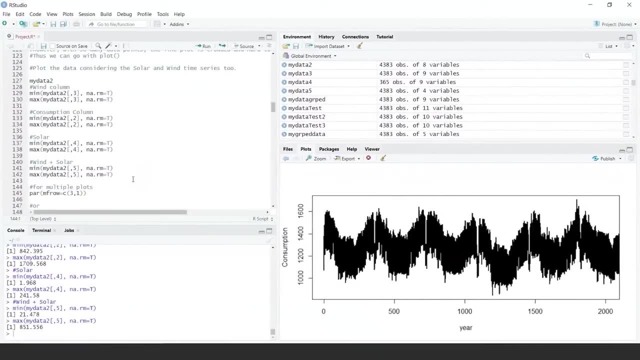 this will be helpful when you would want to plot multiple graphs or give some limits. so that's fine. now for multiple plots. as I said, instead of having one plot, let's plot consumption and wind and solar and try to see a pattern so I can say par function and I will. 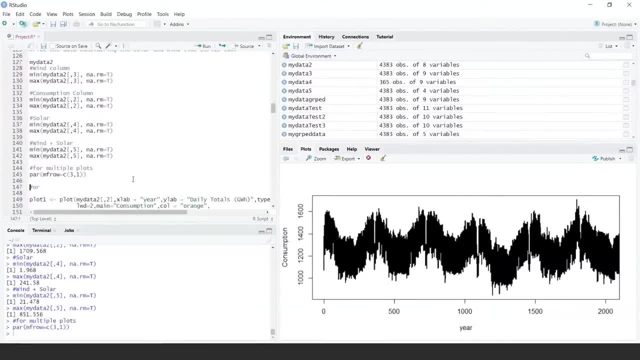 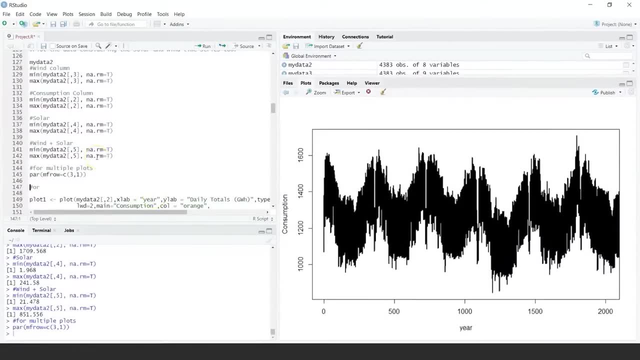 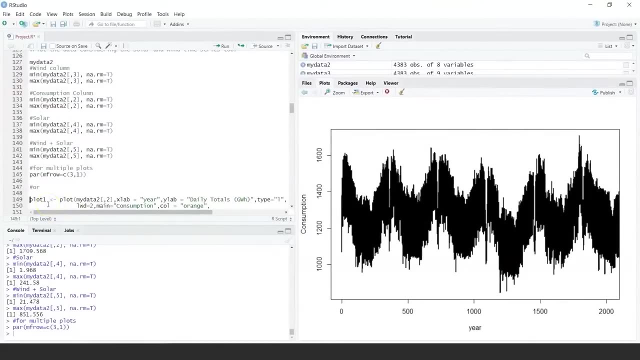 say three rows and one column. so now when I start plotting, you will see, you will have multiple plots in one single window. so let's see how we do it. so here let's look at plot one. so this one is consumption, as we did earlier, and let's look. 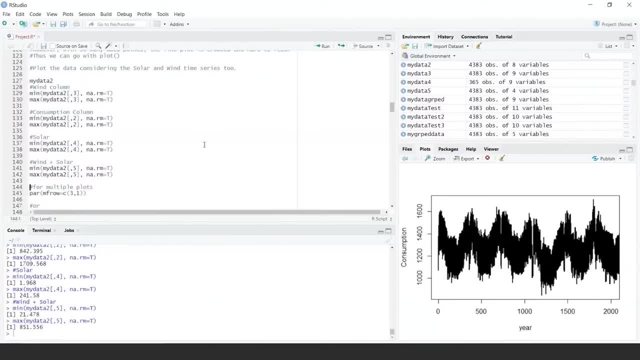 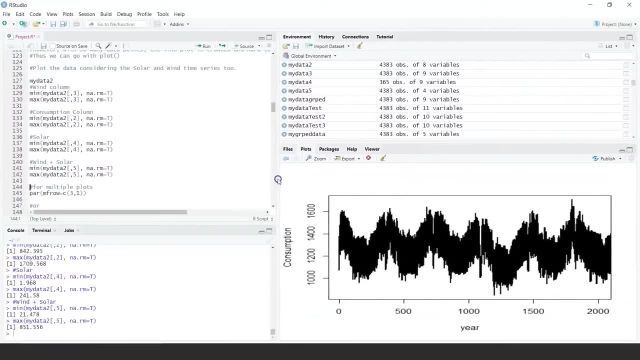 and wind, plus solar minimum and maximum. so this will be helpful when you would want to plot multiple graphs or give some limits. so that's fine. now for multiple plots. as I said, instead of having one plot, let's plot consumption and wind and solar and try to see a pattern. 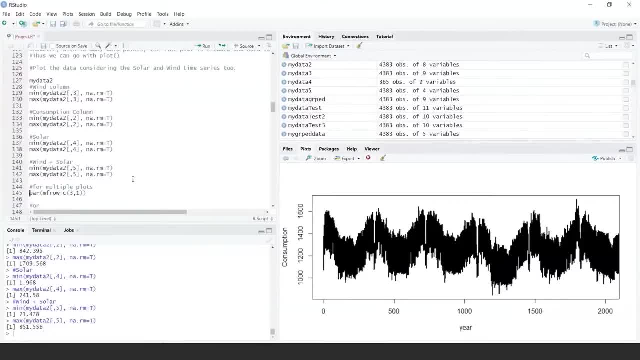 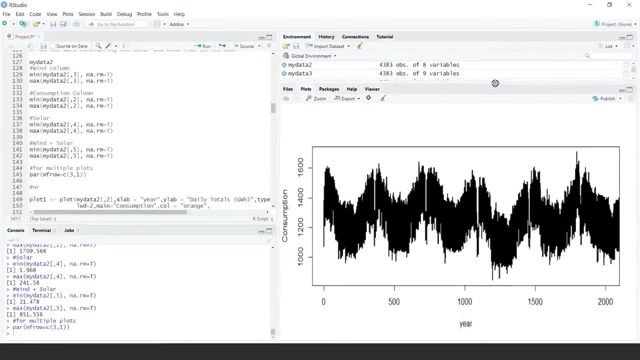 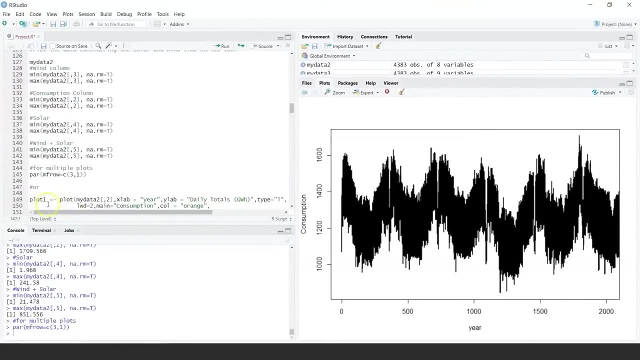 so I can say par function and I will say three rows and one column. so now when I start plotting, you will see, you will have multiple plots in one single window. so let's see how we do it. so here let's look at plot one. so this one is: 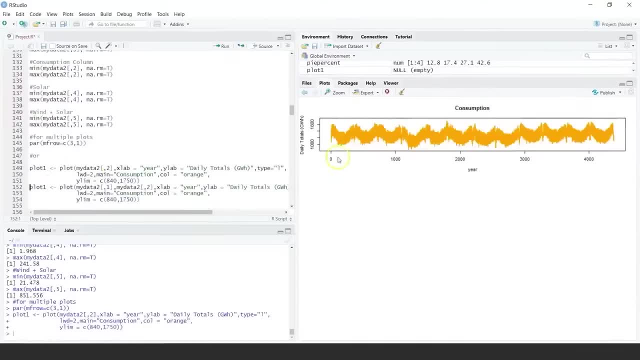 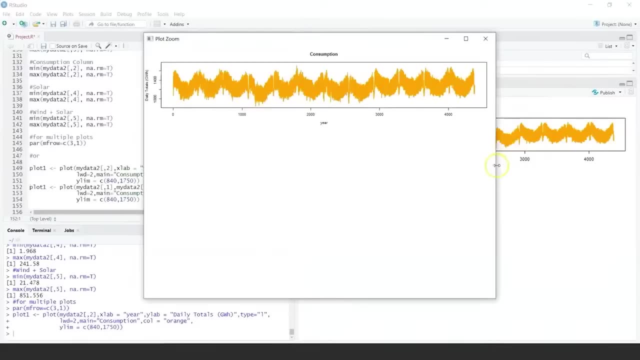 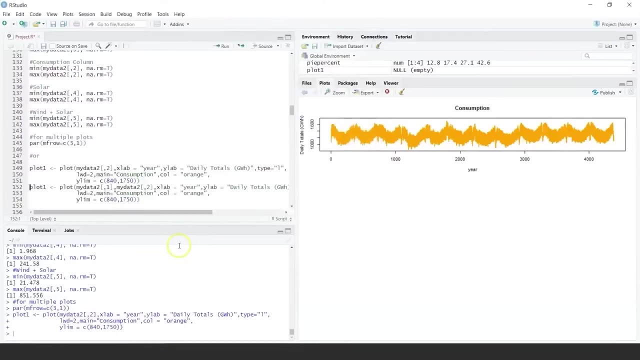 consumption, as we did earlier, and let's look at the data. so that gives me some data. you can always do a zoom and you can look at the data. you can basically expand this graph or you can reduce this graph to see what kind of pattern we have in consumption. 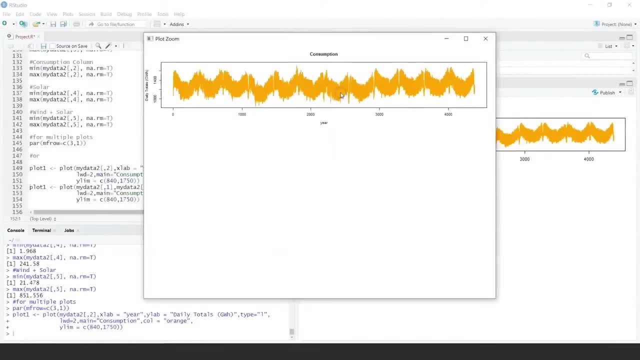 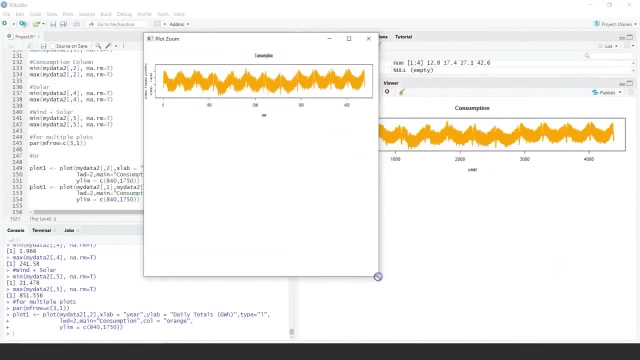 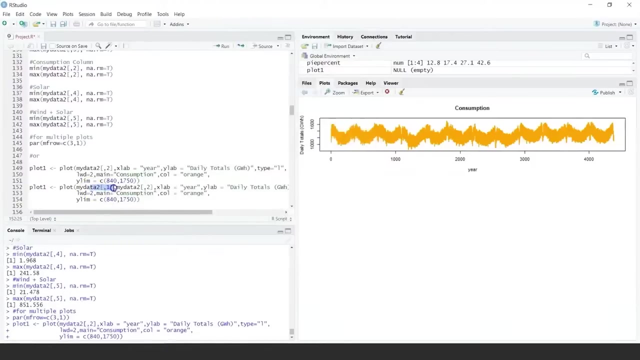 at the data. so that gives me some data. you can always do a zoom and you can look at the data. you can basically expand this graph or you can reduce this graph to see what kind of pattern we have in consumption. similarly, we can basically choose date being. 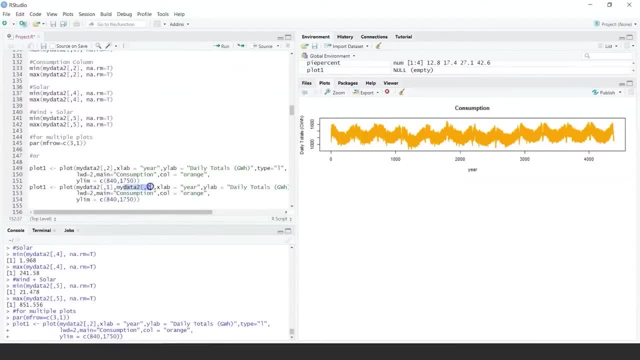 x axis, my consumption being y axis. right, so this is being more specific, because here we have a range, but it really does not give me enough information. so I will basically give x axis, y axis, I will give the name, that is, daily totals, and then I will basically give consumption. 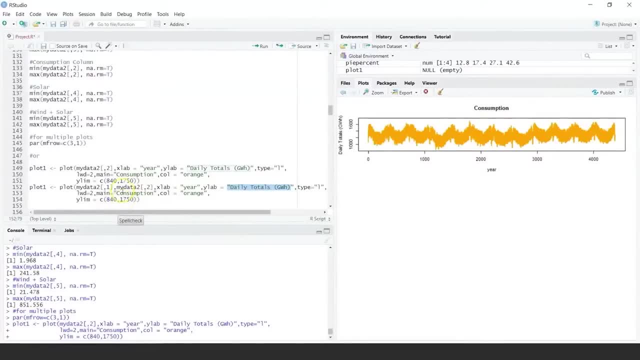 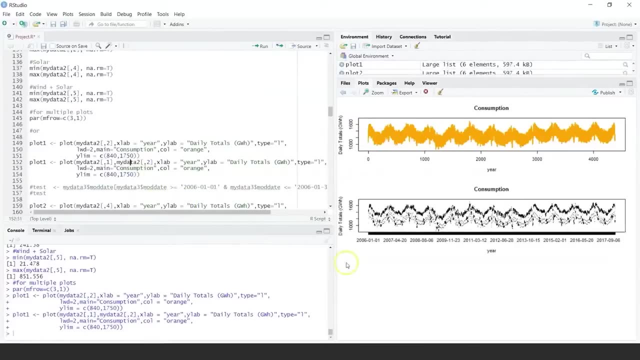 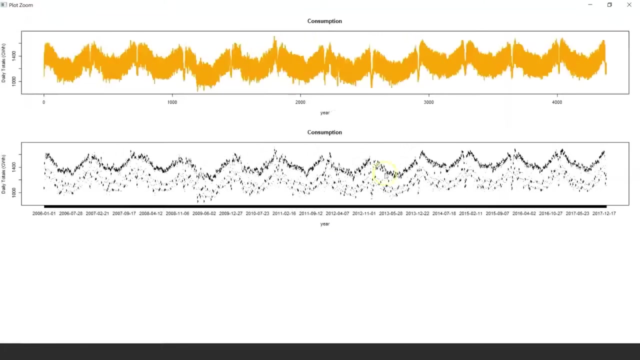 color and y limit, based on my minimum and maximum limits. so let's do this. and now we can look at the data here. so let's see, this data makes a little more meaning because we are looking at the dates and let me do a zoom so it shows me all the dates. 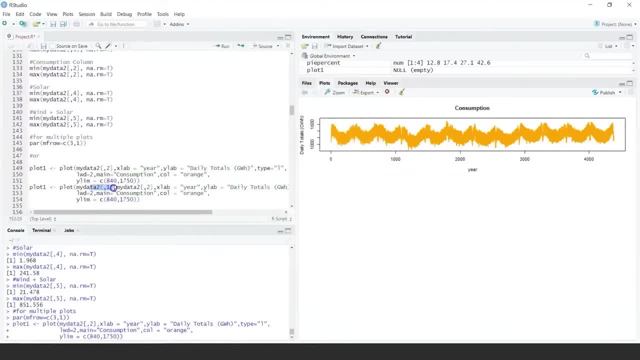 similarly, we can basically choose date being x axis, my consumption being y axis, right? so this is being more specific because here we have a range, but it really does not give me enough information. so I will basically give x axis, y axis, I will give the name that is daily. 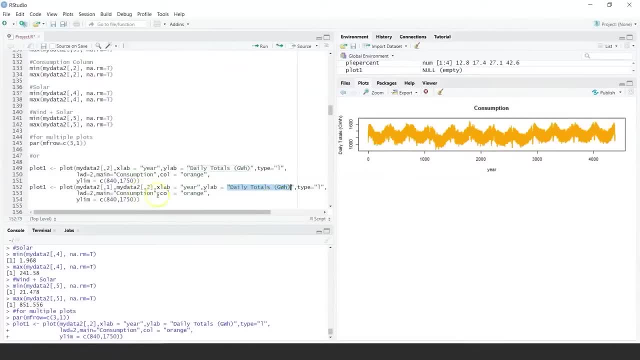 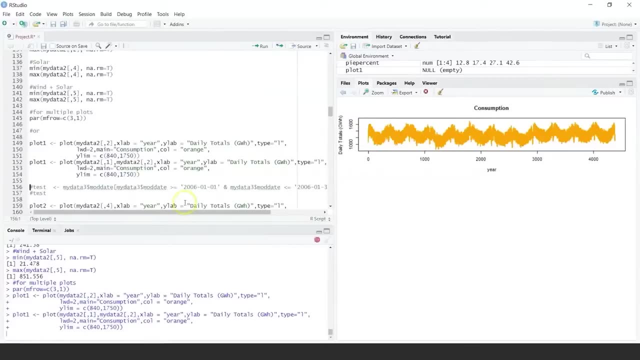 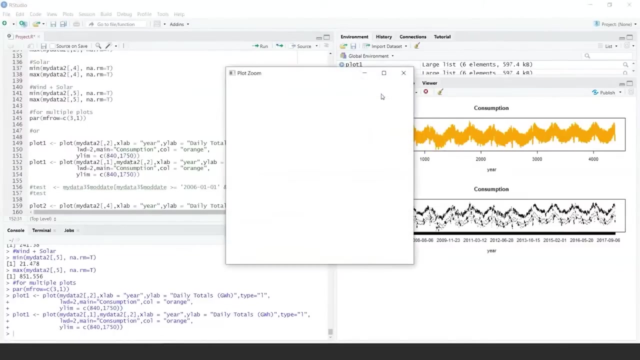 totals and then I will basically give consumption color and y limit based on my minimum and maximum limits. so let's do this, and now we can look at the data here. so let's see, this data makes a little more meaning because we are looking at the dates. 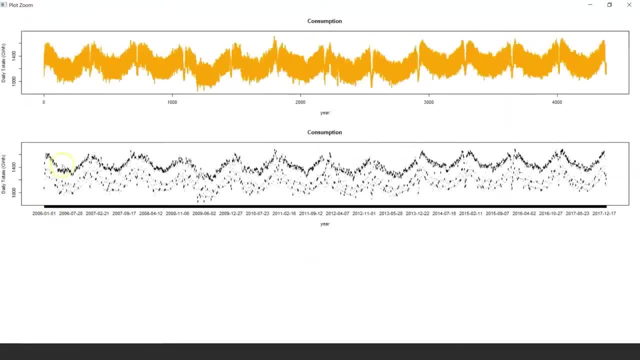 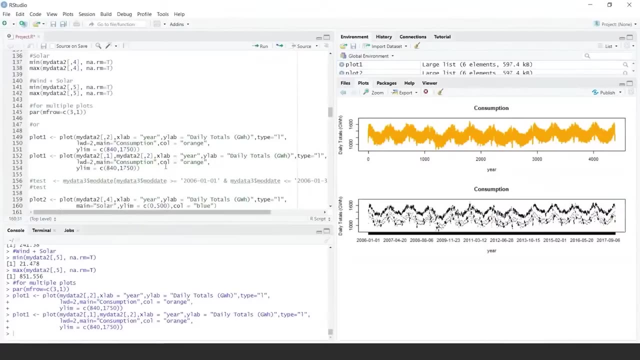 and let me do a zoom. so it shows me all the dates, it shows me the data points, it shows me how the data pattern is changing for consumption. now, this is for consumption, so what we can do is we can also extract specific data. so if you see, here I have done some testing. 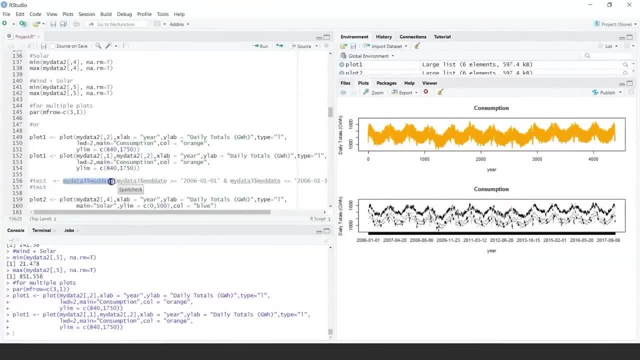 where I am saying, okay, I would want to get a date. specifically, I would want to extract some value. so we are looking at the date column but, if you remember, we did not change the data type. we just change the data type of date column. we extracted year. 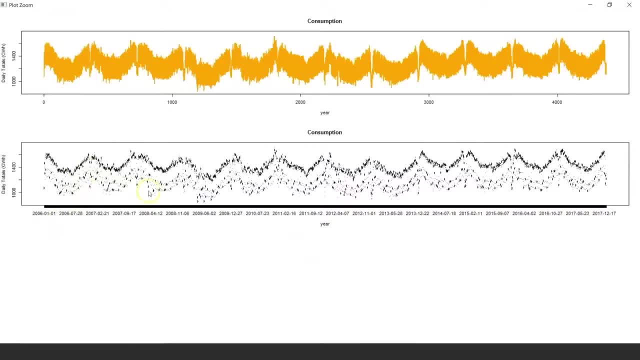 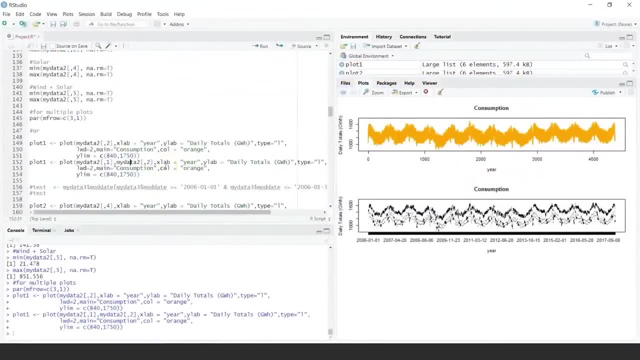 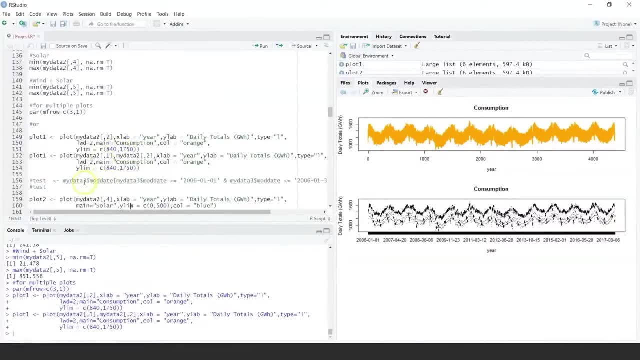 it shows me the data points. it shows me how the data pattern is changing for consumption: now, this is for consumption, so what we can do is we can also extract specific data. so if you see, here I have done some testing where I am saying: okay, I would want to. 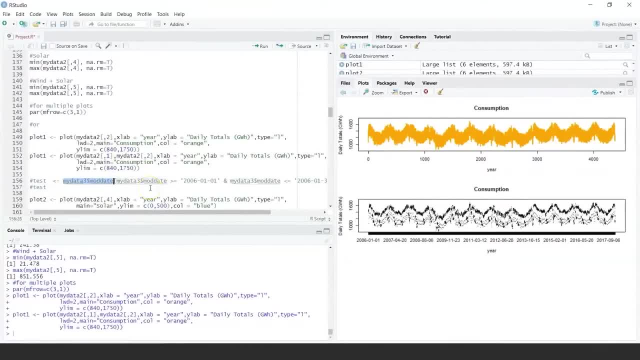 get a date specifically, I would want to extract some value. so we are looking at the date column but if you remember, we did not change the data type. we just change the data type of date column. we extracted year, month out of it. it would be good if we can. 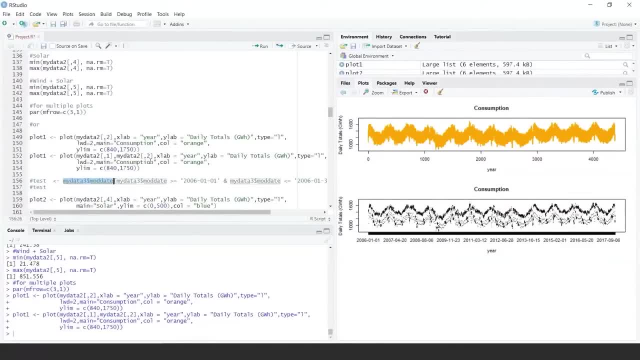 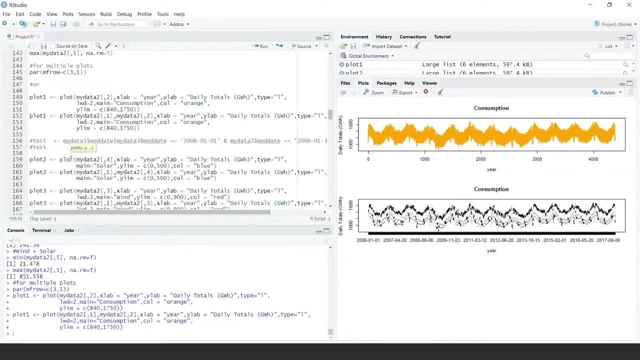 convert a column into date time format and put that in our data frame. now let's look at the plot 2. this is mainly for your column, which should be consumption and wind and solar. so here I see it is solar data and I can plot this one. 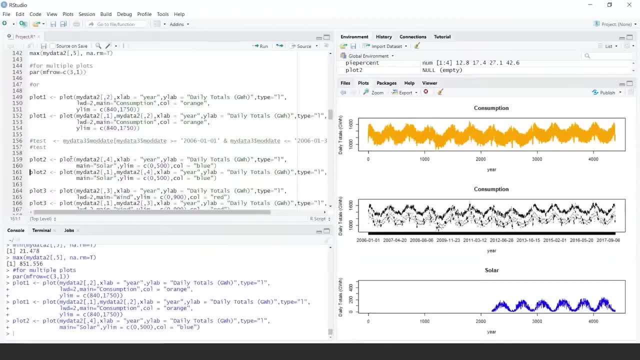 to see how it looks like and that tells me. from 2006 onwards we have some pattern. I can be more specific where I say I would be giving date and then the column for solar x axis, y axis: what is the type, what is the y limit and what? 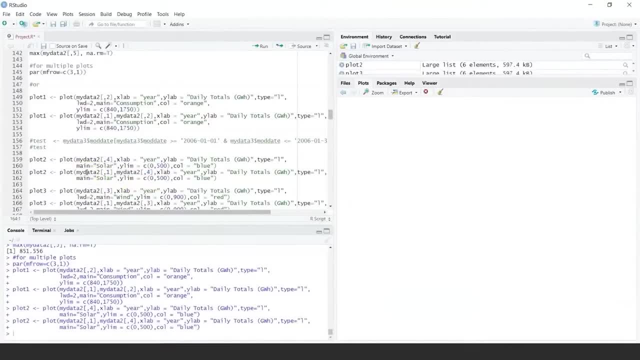 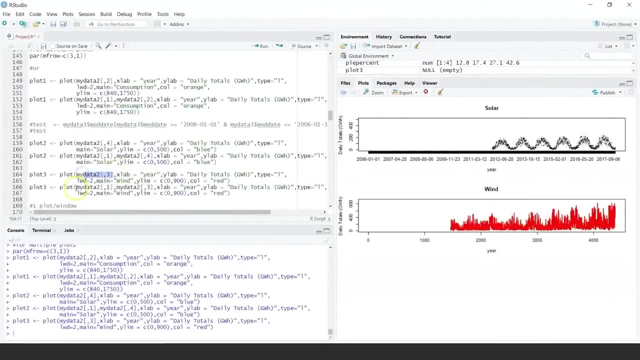 is the color. it is always good to specify your x and y axis given name rather than let it automatically pick up. now this makes more meaning because it shows me some dates. similarly we can do for wind. so either you do it just by giving the column or you give your. 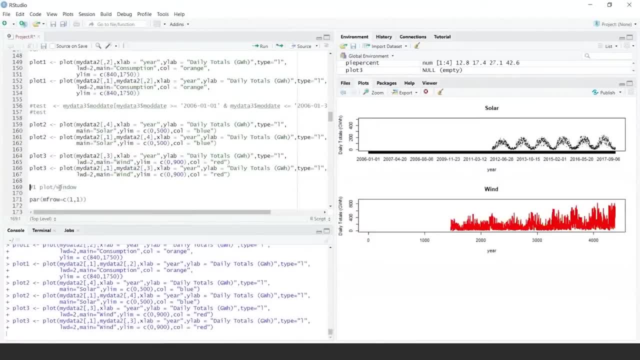 x and y axis. so let's look at this one and this shows me the data. so we can choose plot 3, this one, we can choose plot 2, we can choose plot 1 and we can put all that data in one graph. so that's when you are putting in multi. 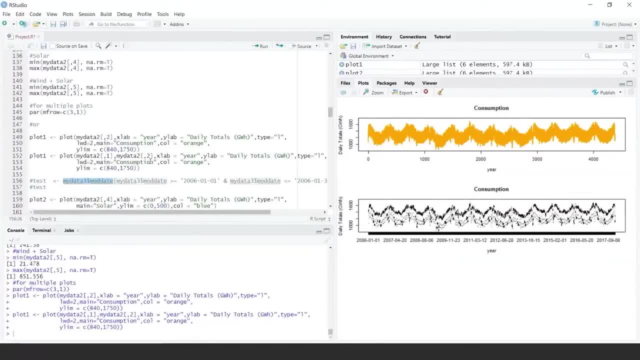 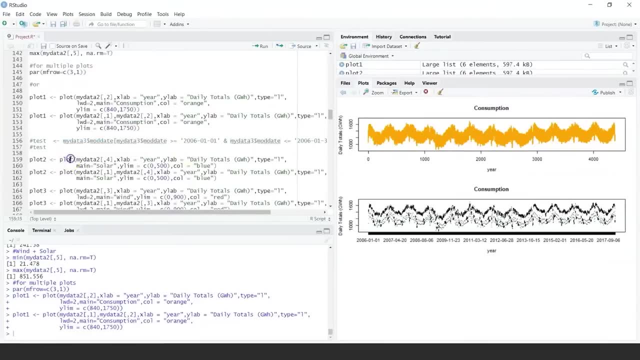 month out of it. it would be good if we can convert a column into date time format and put that in our data frame. now let's look at the plot 2. this is mainly for your column, which should be consumption and wind and solar. so here I 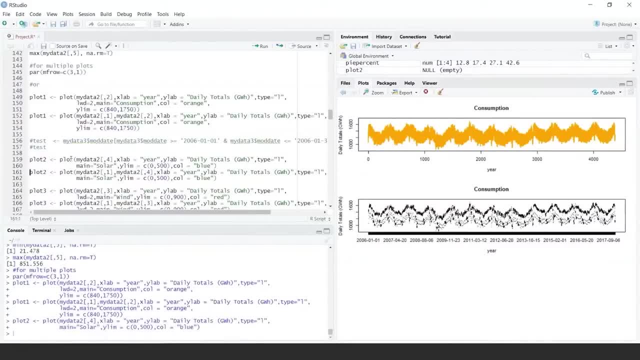 see, it is solar data and I can plot this one to see how it looks like and that tells me from 2006 onwards. we have some pattern. I can be more specific where I say I would be giving date and then the column for solar x axis, y axis. 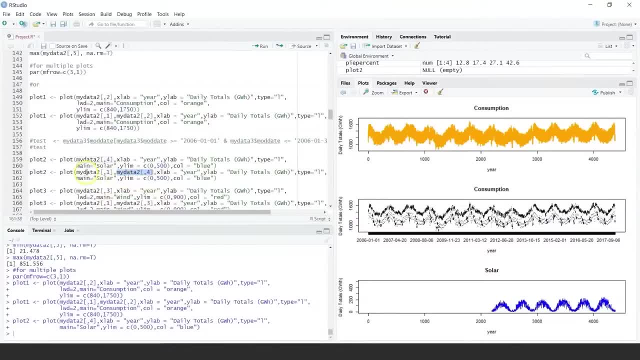 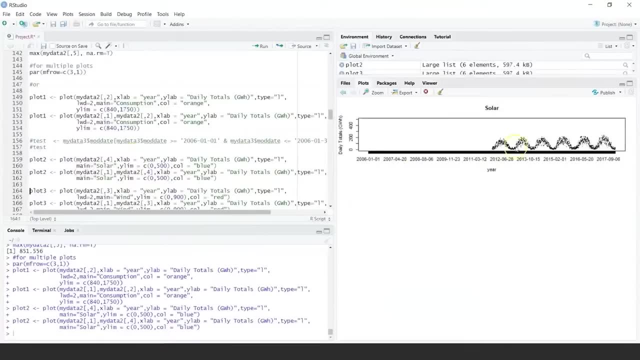 what is the type, what is the y limit and what is the color? it is always good to specify your x and y axis given name rather than let it automatically pick up now. this makes more meaning because it shows me some dates. similarly, we can do for wind. 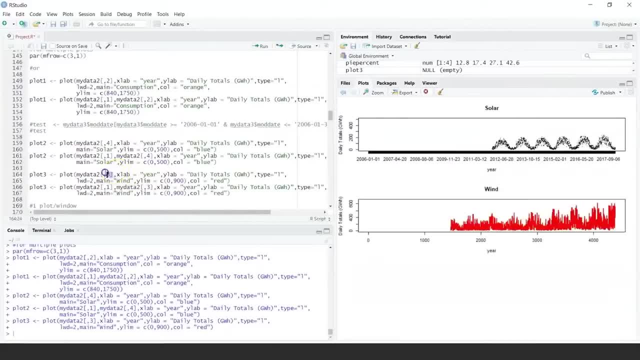 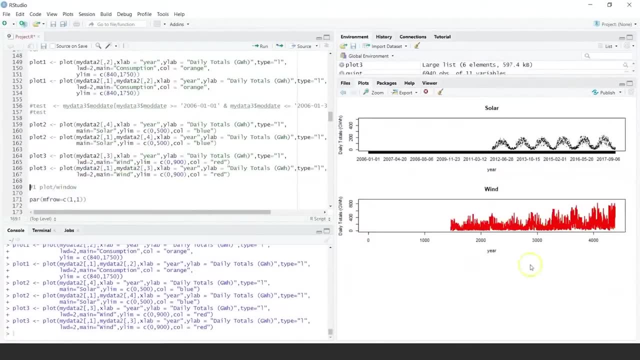 so either you do it just by giving the column or you give your x and y axis. so let's look at this one and this shows me the data. so we can choose plot 3, this one, we can choose plot 2. we can choose plot 1. 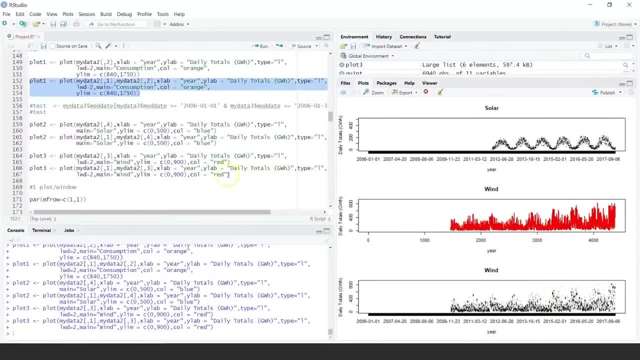 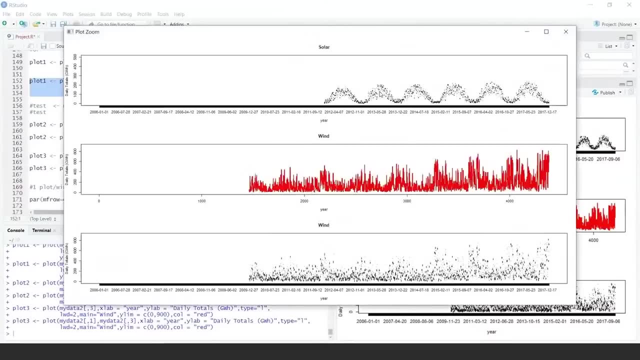 and we can put all that data in one graph. so that's, when you are putting in multi plots in one particular graph, you can always do a zoom, you can always look at the data right, and this is usually useful to look at the pattern. what kind of pattern. 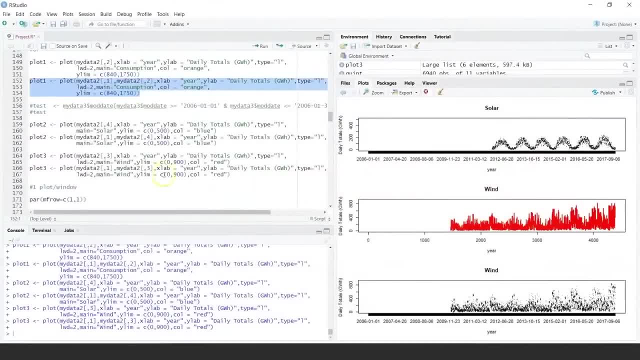 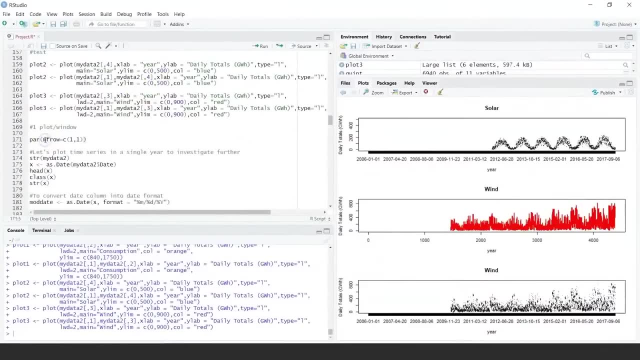 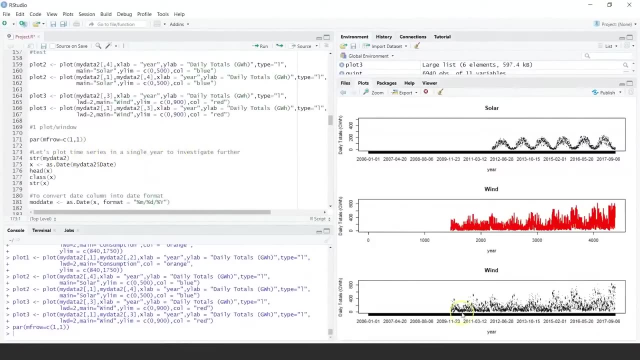 we see what data we have, and so on. now moving forward. so we have seen how you are creating these plots all in one window. let me reset this back to one plot per window and let's basically plot time series in a single year. so what we have. 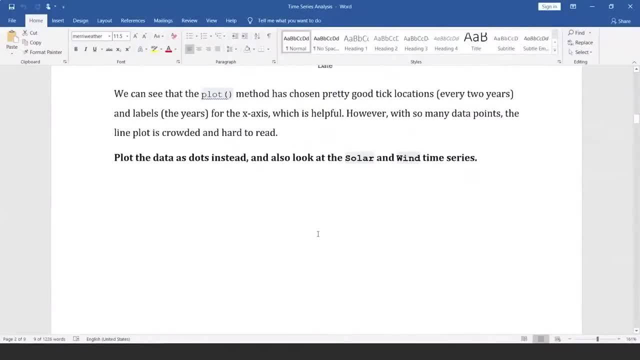 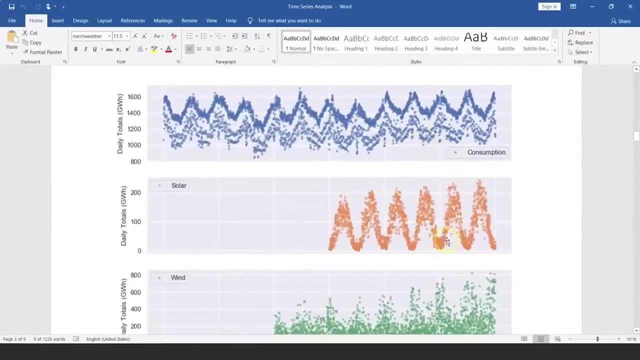 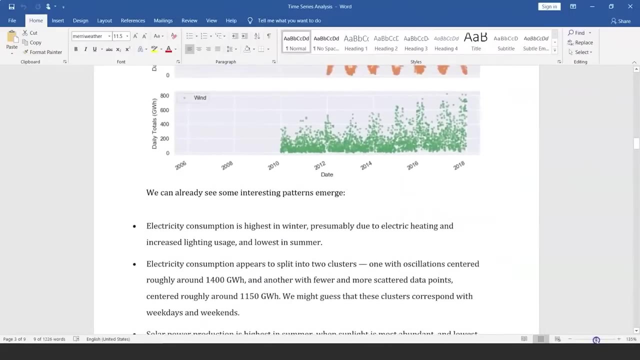 seen is that when you look at the plot method, it was quite crowded. then we looked at solar and wind and if you compare that you will see your consumption pattern, your solar pattern, your wind pattern and basically we can see from this particular data some kind of pattern. so electricity: 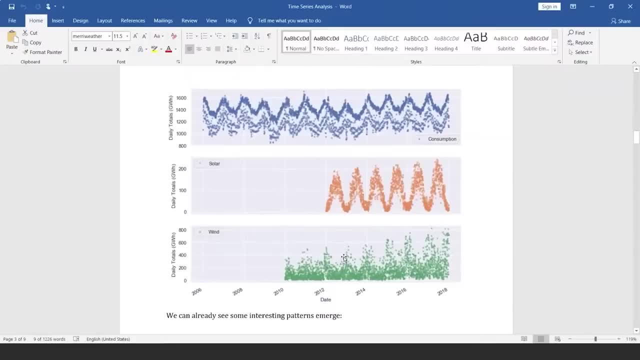 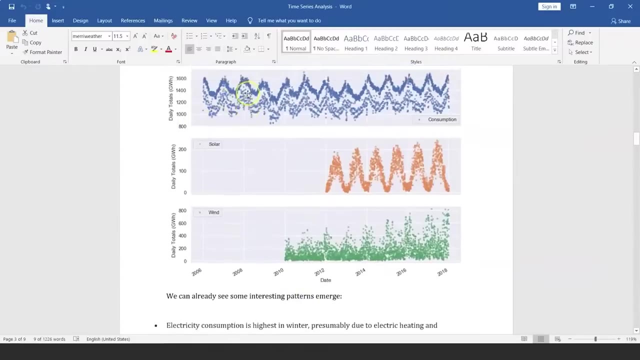 consumption is highest in the winter, where we will see what is the consumption: is it highest in winter or is it in summer? we can see that by breaking a year further into months. we can see that, but we see a pattern which goes for every year or every two years. 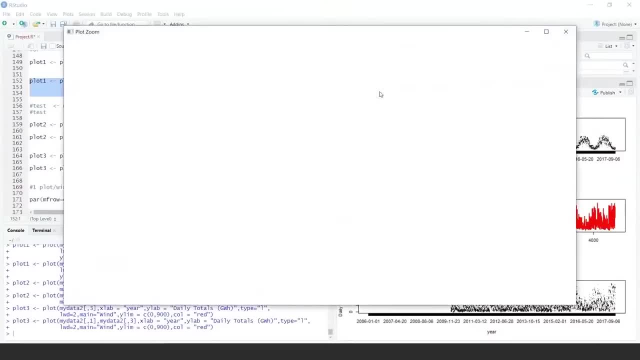 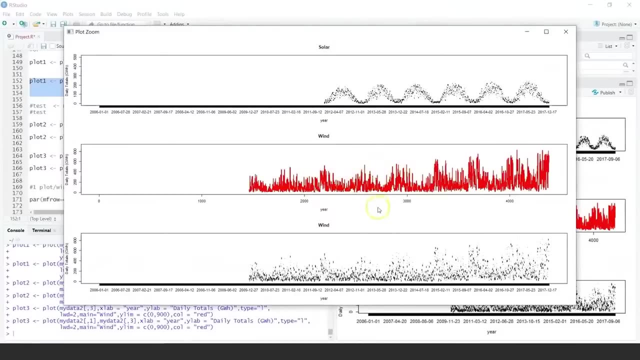 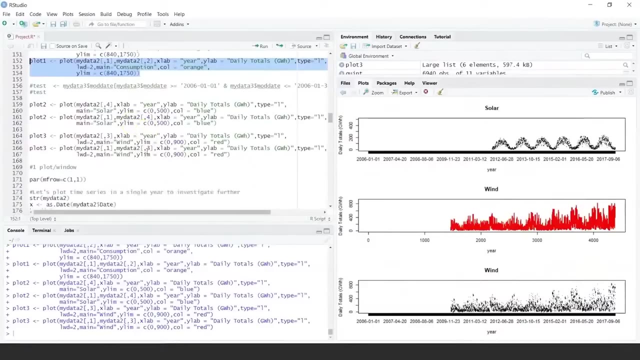 plots in one particular graph. you can always do a zoom, you can always look at the data right- and this is usually useful- to look at the pattern, what kind of pattern we see, what data we have, and so on. now moving forward, so we have seen how you are creating. 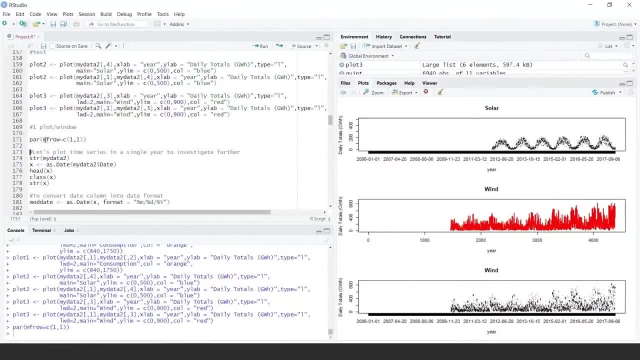 these plots all in one window. let me reset this back to one plot per window and let's basically plot time series in a single year. so what we have seen is that when you look at the plot method, it was quite crowded. then we looked at solar and 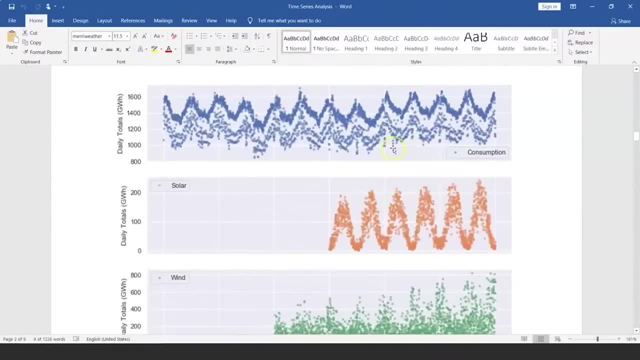 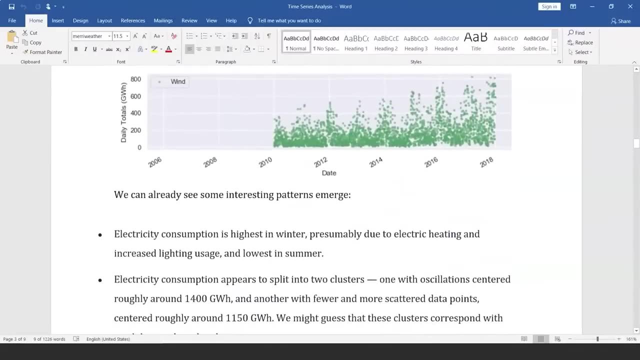 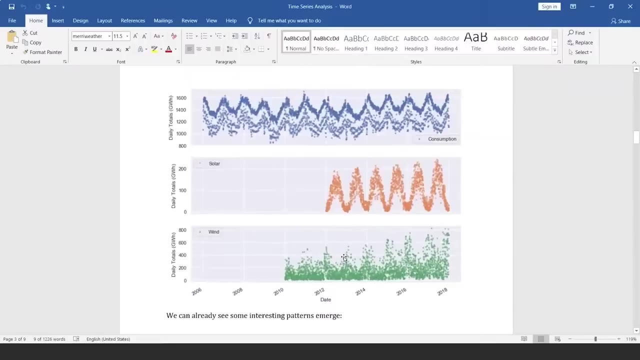 wind and if you compare that, you will see your consumption pattern, your solar pattern, your wind pattern and basically we can see from this particular data some kind of pattern. so electricity consumption is highest in the winter, where we will see what is the consumption: is it highest in winter or is it in summer? we can 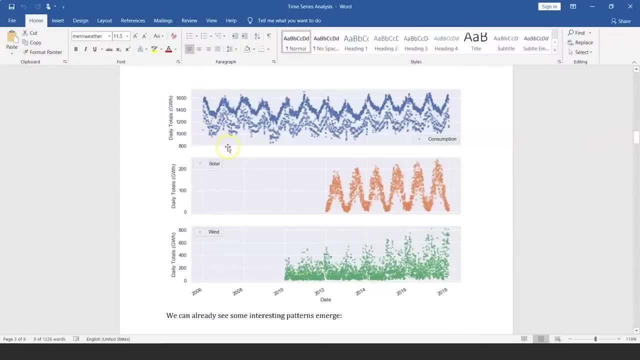 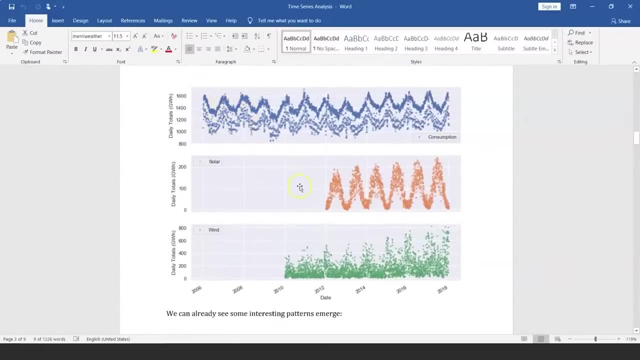 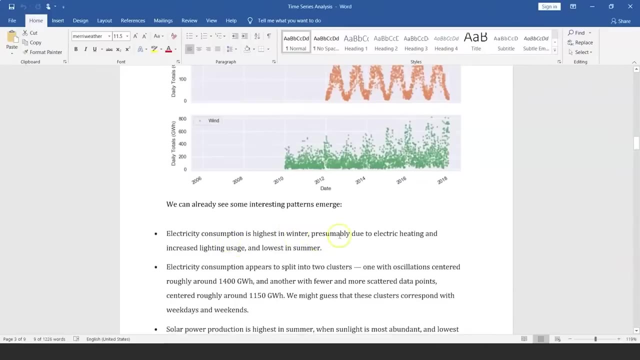 see that by breaking a year further into months we can see that. but we see a pattern which goes for every year or every two years, being highest at a particular point of time and then it drops down. so electricity consumption is highest in winter and that might be due. 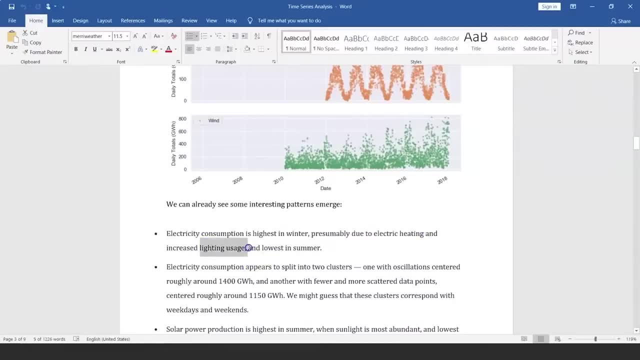 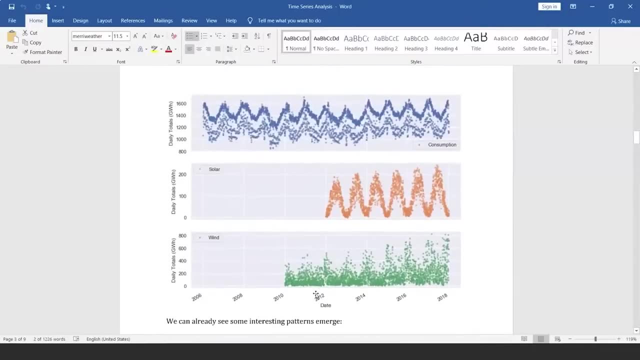 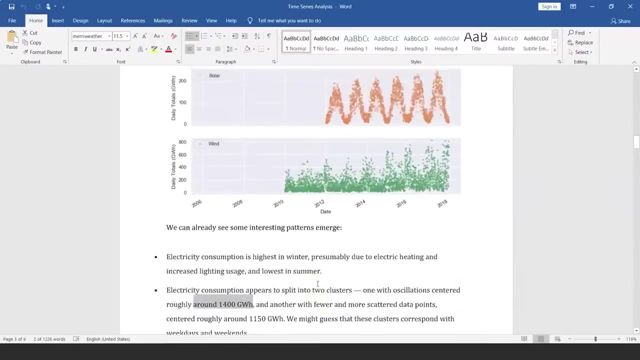 to electrical heating and increased lighting usage, and lowest in summer. now, when you look at electricity, consumption appears to split into two clusters. we can always look at the consumption one with oscillation centered roundly around 1400 gigawatts. so you can always look at. 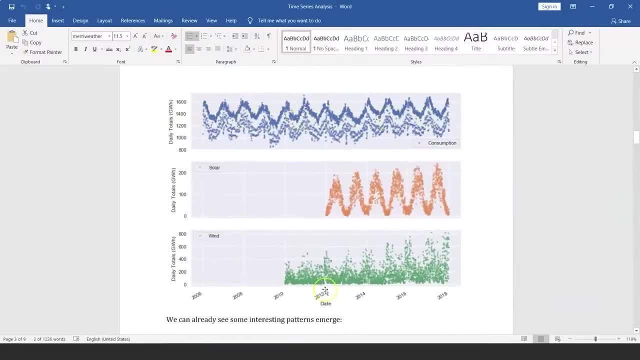 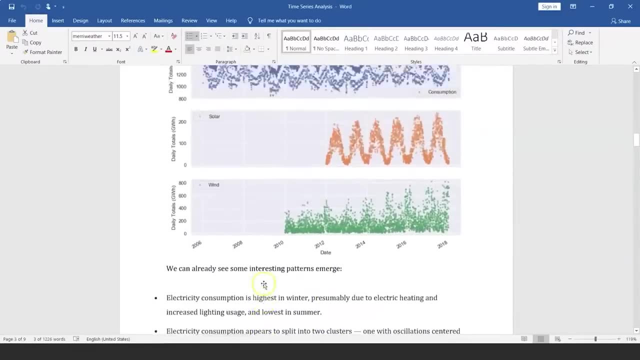 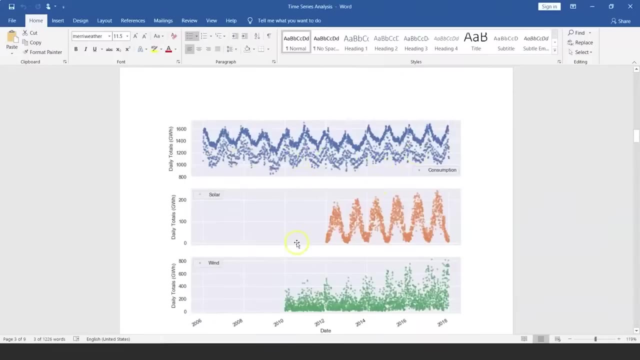 1400 gigawatts and you see all the values here which are in that particular consumption. another with fewer and more scattered data points, centrally roughed around 1150. so if you really expand this, you can see you will have lot of data points at this point. 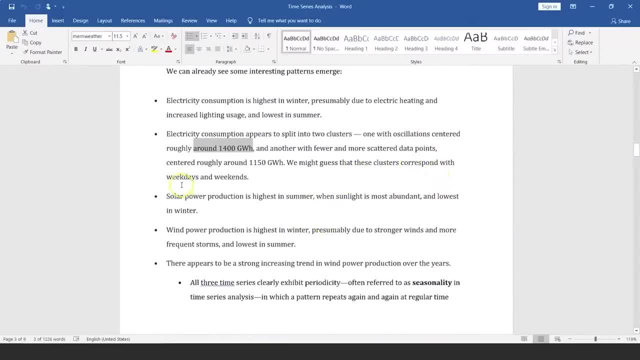 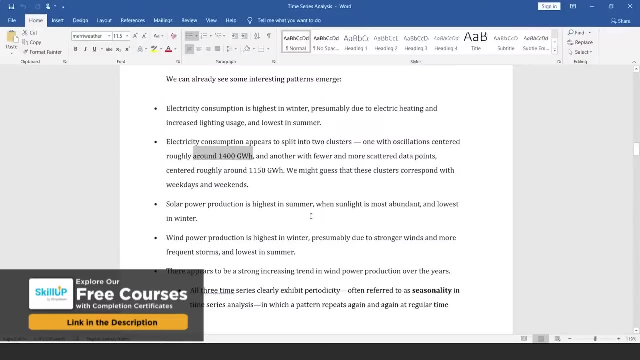 now we might guess that these clusters correspond with week days and weekends, which we can see if you break that data into yearly, monthly, weekly and so on. now, if you look at solar production, that is highest in summer, when sunlight is most abundant, and lowest in winter. so obviously, 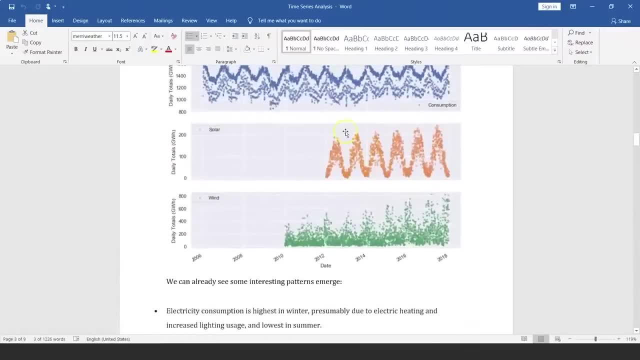 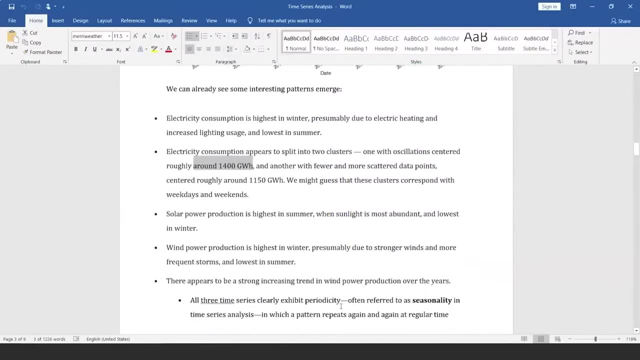 when you are making or gathering some insights, when you are looking at the data, you are also using your domain knowledge, your business knowledge, your you know knowledge of business to understand how this goes. if you look at wind power production, that's again highest in winters and drops down in summer. 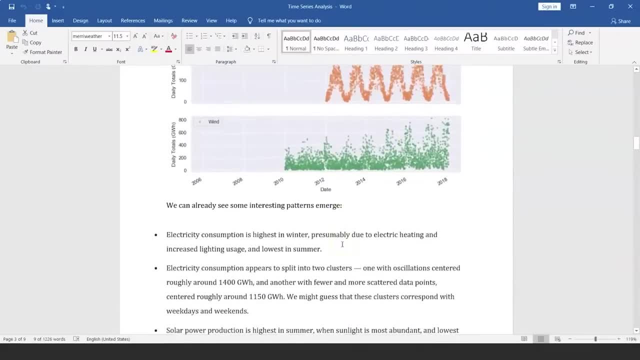 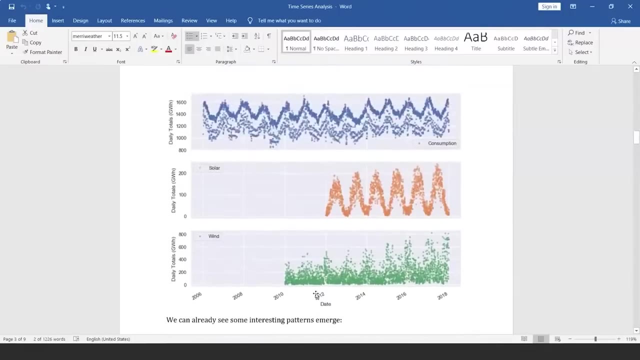 being highest at a particular point of time and then it drops down. so electricity consumption is highest in winter and that might be due to electrical heating and increased lighting usage and increased temperature in summer. now, when you look at electricity consumption appears to split into two clusters. we can 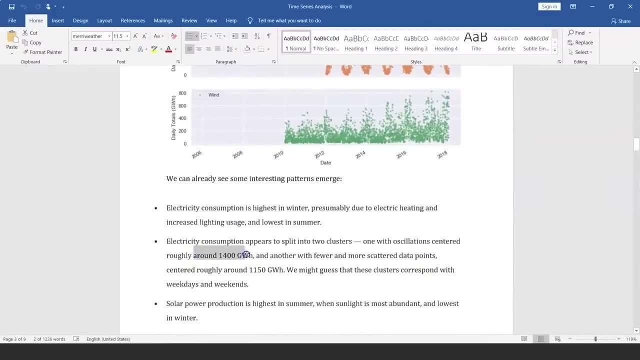 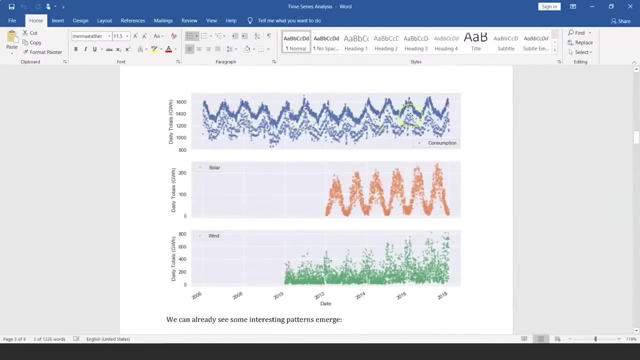 always look at the consumption, one with oscillation centered roundly around 1400 gigawatts. so you can always look at 1400 gigawatts and you see all the values here which are in that particular consumption. another with fewer and more scattered data. 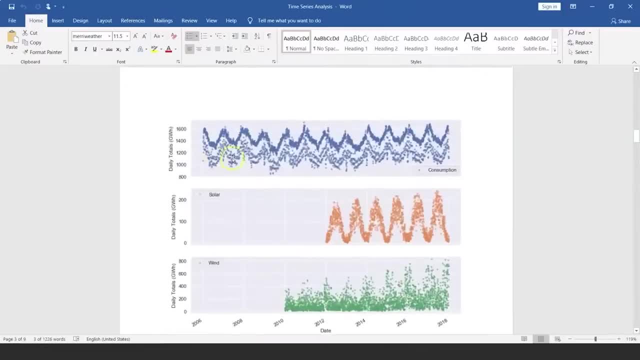 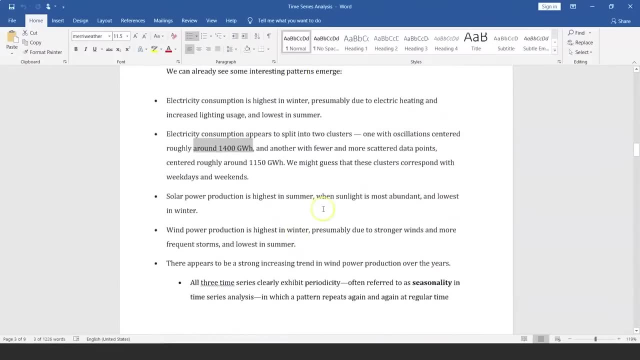 points, centrally roughed around 1150. so if you really expand this, you can see you will have lot of data points. at this point now we might guess that these clusters correspond with weekdays and weekends, which we can see if you break that data into yearly, monthly, weekly and so on. 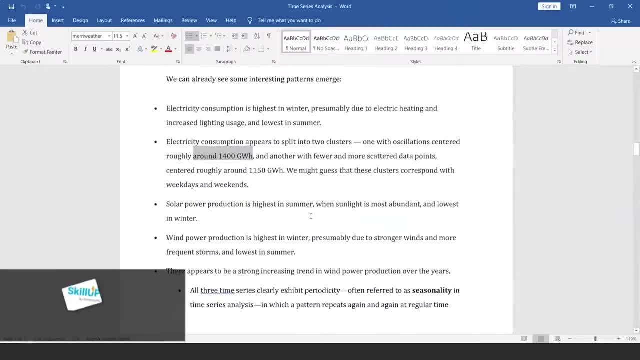 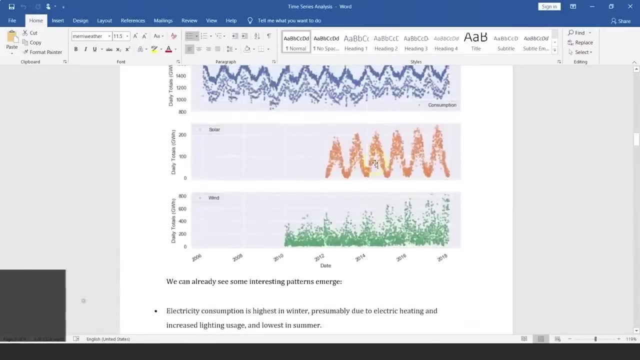 now, if you look at solar production, that is highest in summer, when sunlight is most abundant, and lowest in winter. so obviously, when you are making or gathering some insights, when you are looking at the data, you are also using your domain knowledge, your business knowledge, your- you know- knowledge of business to 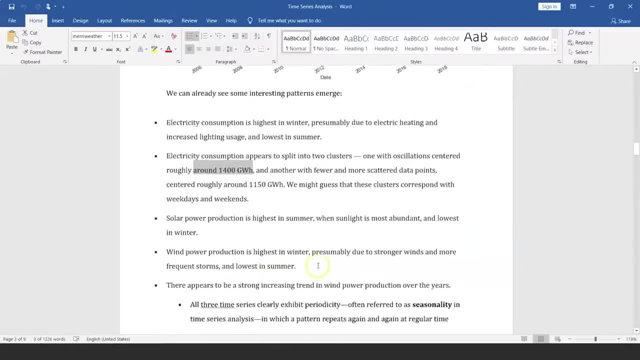 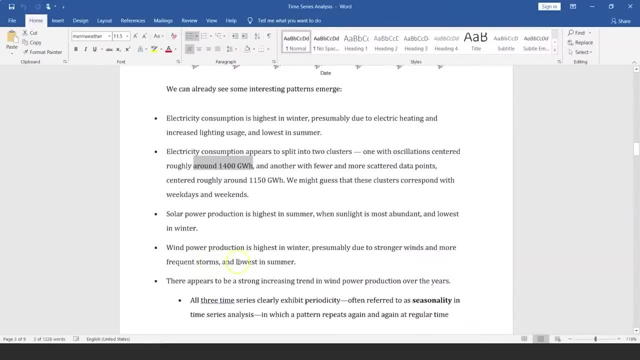 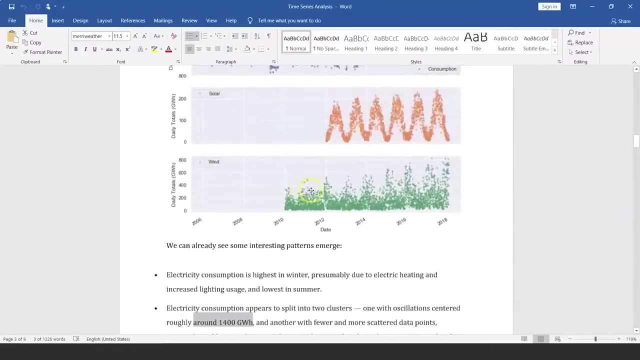 understand how this goes. if you look at wind power production, that's again highest in winters and drops down in summer- so due to stronger winds and more frequent storms- and lowest in summer. so there is some kind of increasing trend in wind power production over years which we can see here. 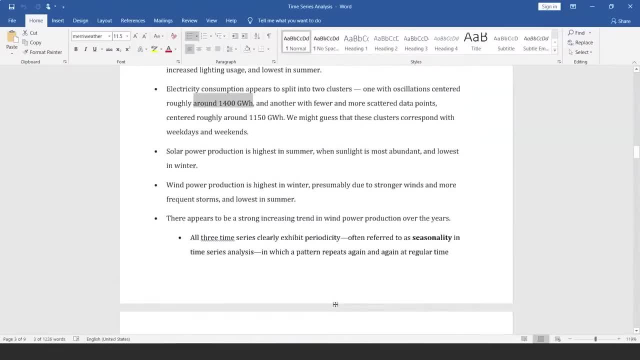 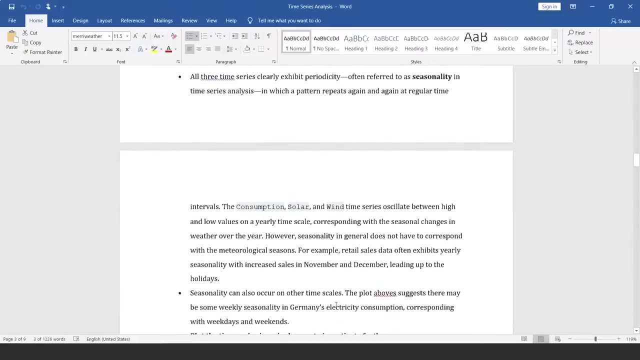 over the years and all the time series data. what we are looking at is referring or showing us some kind of seasonality, that is, we are looking at seasonality in which a pattern is repeating again and again at regular times, at regular intervals. so if you look at 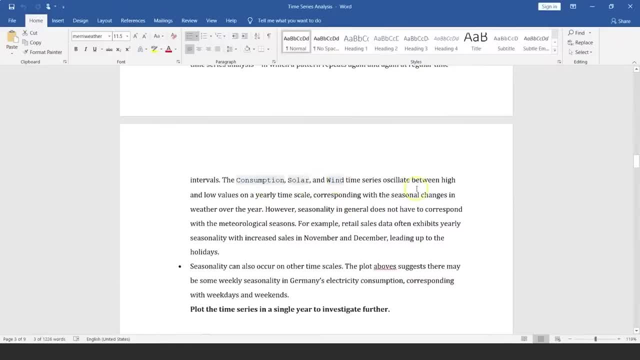 consumption, solar and wind- time series that oscillates between high and low values on a yearly time scale which we can break down and see. i'll show you that it corresponds with the seasonal changes in weather over the year. so seasonality does not have to correspond with. 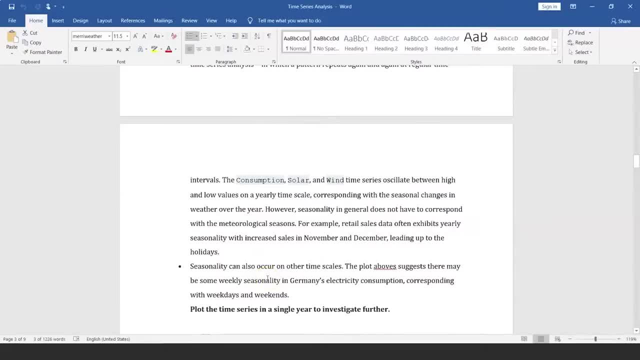 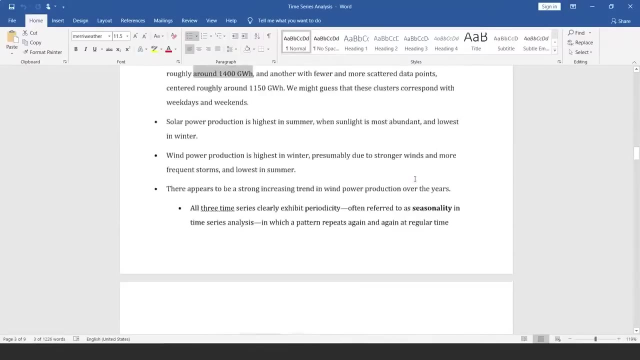 hydrological reasons, for example. if you look at retail sales data, that will show you yearly seasonality, with increased sales in particular months. so seasonality, when we say, can occur on other time scales. so the plots, what we are seeing here, they are fine, but if you look at those plots, 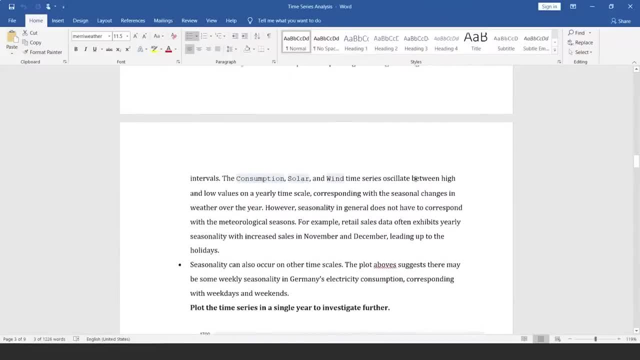 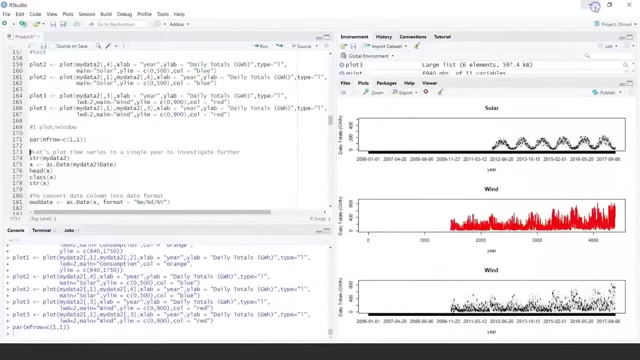 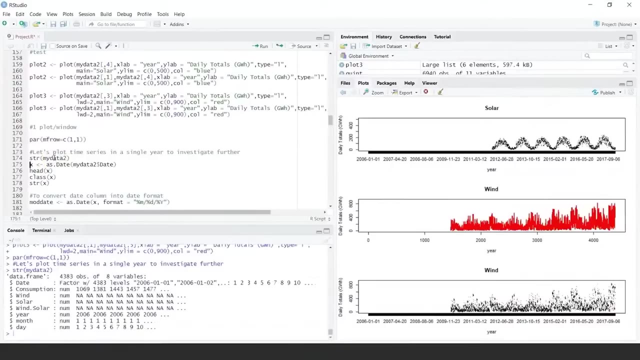 they might show some kind of weekly seasonality also, so in your consumption, corresponding to week days and week ends. so let's plot for one single year. now, how do i do that? so? first is, i will look at my data too. that shows me the structure it shows. 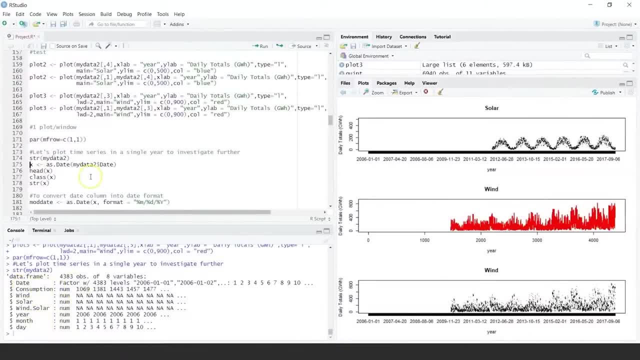 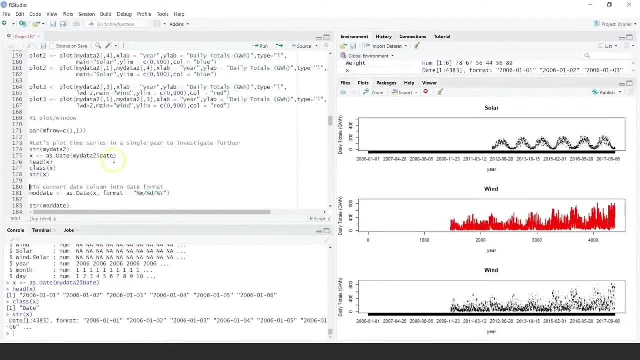 me date, which is factor, other columns which are all numerics. now, like we did earlier, i'll repeat this step where i'm going to convert the date column into date type: look at head of it, look at class of it, look at the structure of it, right and then 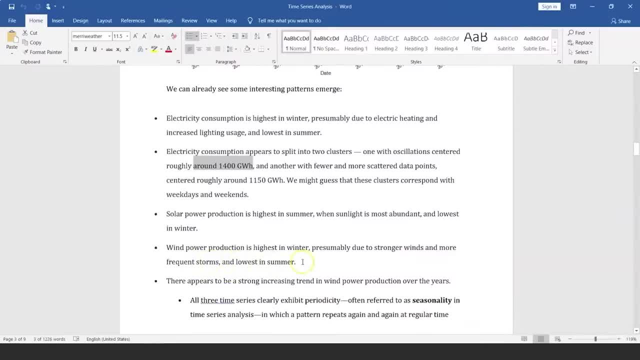 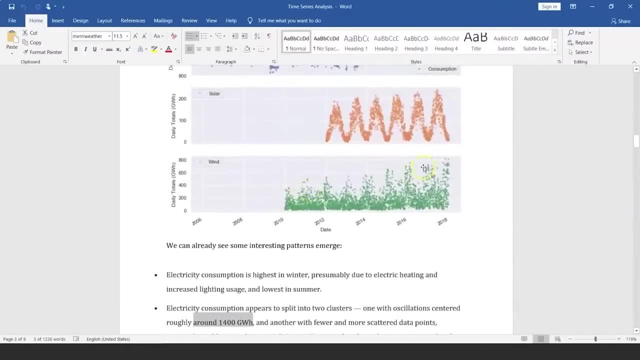 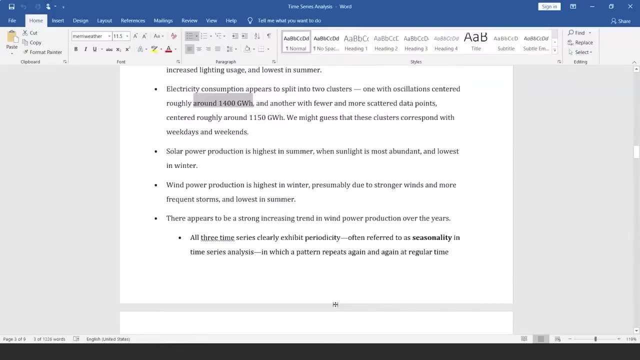 so due to stronger winds and more frequent storms and lowest in summer. so there is some kind of increasing trend in wind power production over years which we can see here over the years and all the time series data. what we are looking at is referring or showing us some kind of seasonality. 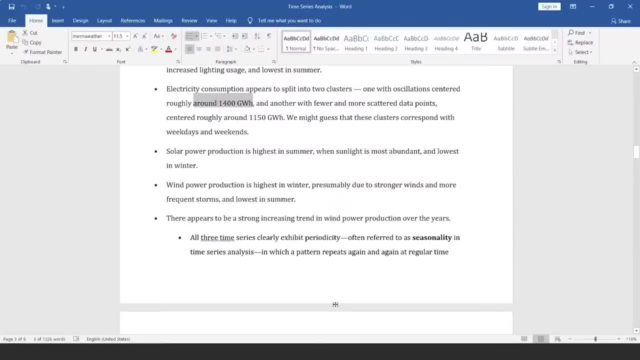 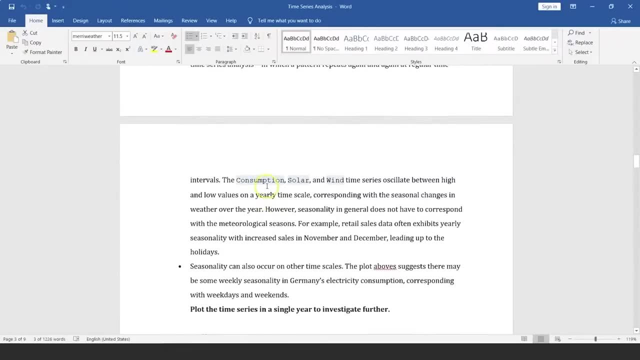 that is, we are looking at seasonality, in which a pattern is repeating again and again at regular times, at regular intervals. so if you look at consumption, solar and wind time series that oscillates between high and low values on a yearly time scale which we can break down and see, I will show you that. 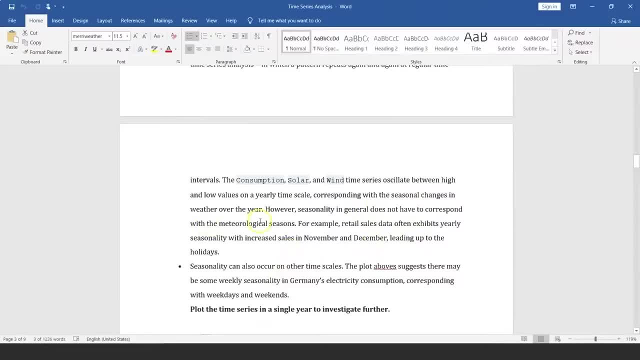 it corresponds with the seasonal changes in weather over the year. so seasonality does not have to correspond with meteorological reasons. for example, if you look at retail sales sales data, that will show you yearly seasonality, with increased sales in particular months. so seasonality when we say 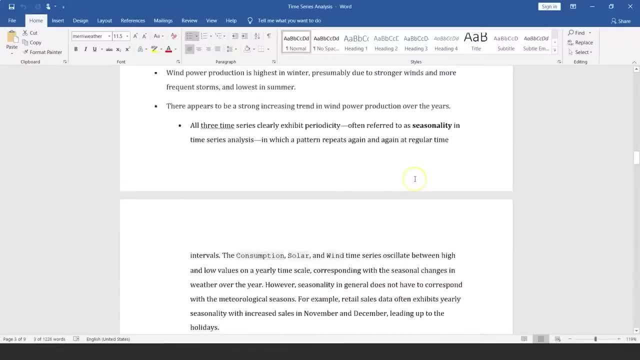 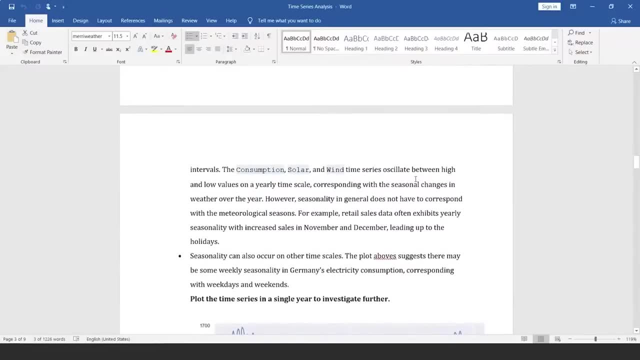 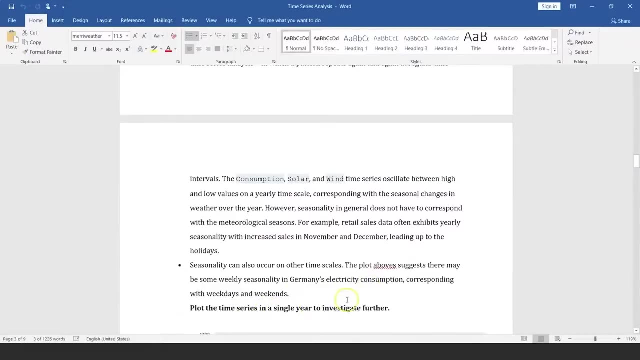 can occur on other time scales. so the plots, what we are seeing here, they are fine, but if you look at those plots they might show some kind of weekly seasonality also, so in your consumption, corresponding to week days and weekend. so lets plot for one single year. 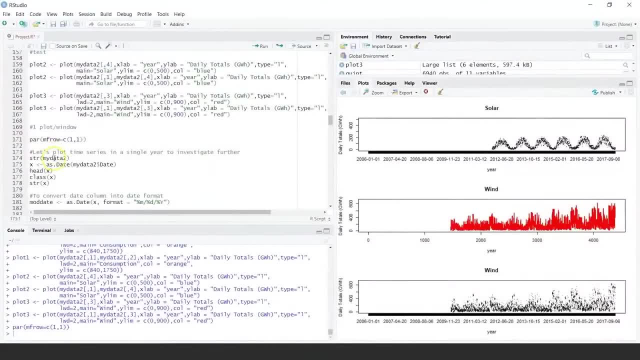 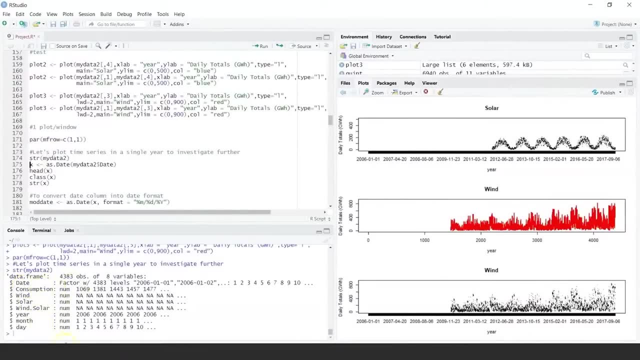 now, how do I do that? so first is, I will look at my data too. that shows me the structure. it shows me date, which is factor, other columns which are all numerics. now, like we did earlier, I will repeat this step where I am going to convert the date column into: 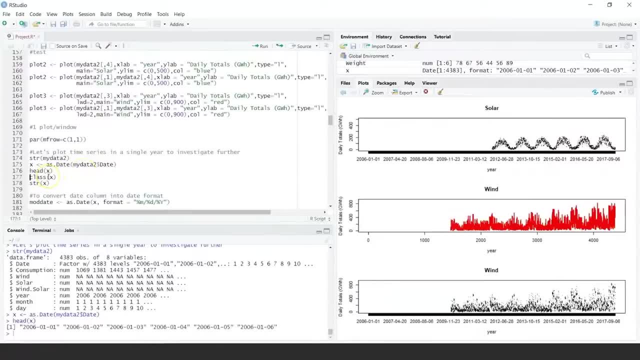 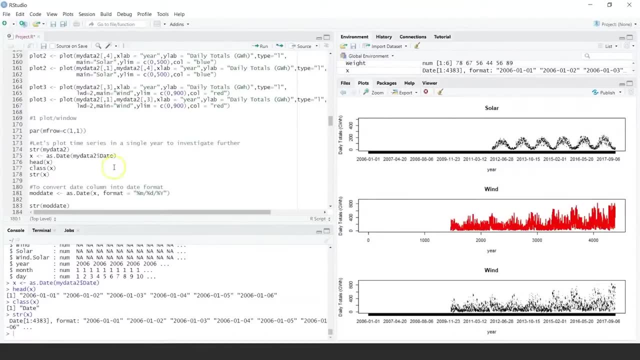 date type, look at head of it, look at class of it, look at the structure of it. right, and then what I want to do is I want to add this to my data frame, so I will create a variable called mod data, and this one will have as data 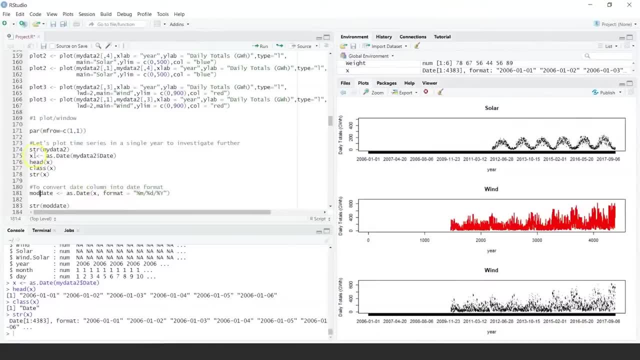 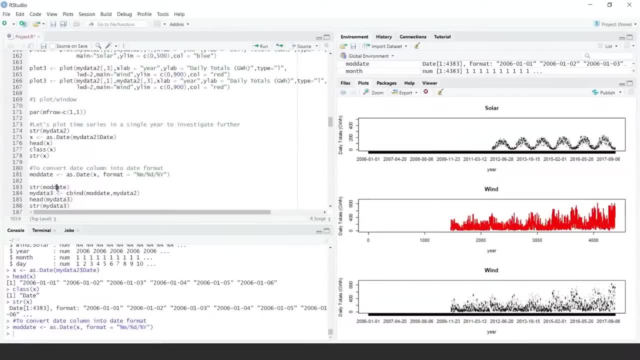 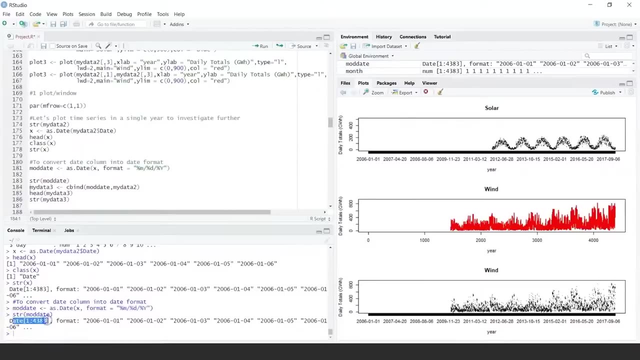 and I am formatting the value of x, which is date time, into month, day and year. so lets do that. and now you look at the mod data which I created like modified data. so this is the format I have. it is in date type, if you carefully see here. 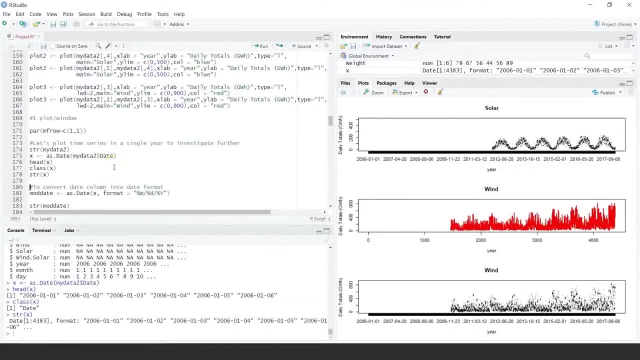 what i want to do is i want to add this add to my data frame. so i will create a variable called mod data and this one will have as data and i'm formatting the value of x, which is date, time, into month, day and year. so let's do that and 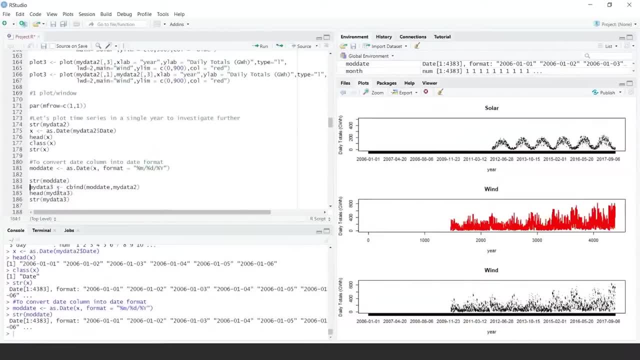 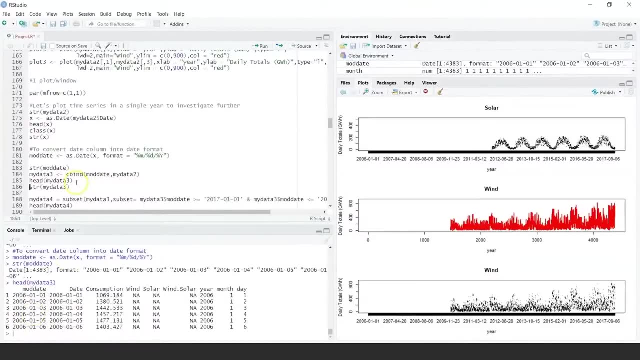 now you look at the mod data which i created like modified data. so this is the format i have. it is in date type, if you carefully see here, and then i can look at the head of it. so it says me: mod data. now we are. what we did here is: 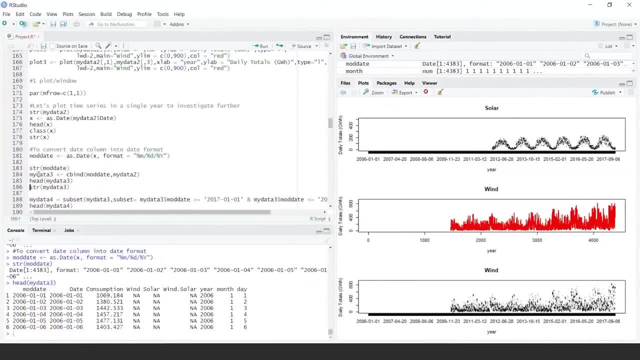 when i said my data 3, so my data 3, we did a c bind and i did a mod data which is going to add this column to my other columns of my data 2. so my new data frame is my data 3. let's look at the structure of it. 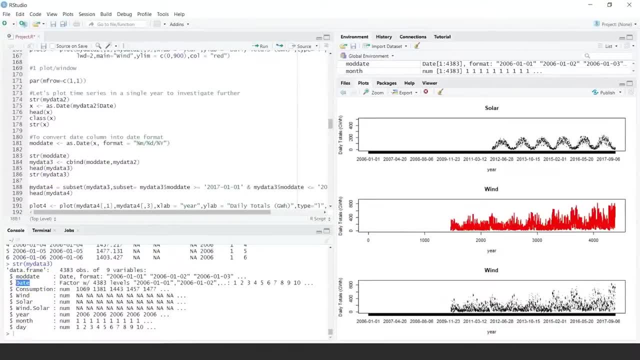 and you see, there is this date column. i can delete it. i can remove it, i can let it be right. so that depends on our choice. might be we want to. once our analysis done, we want to remove the mod data right so we can keep both of them. 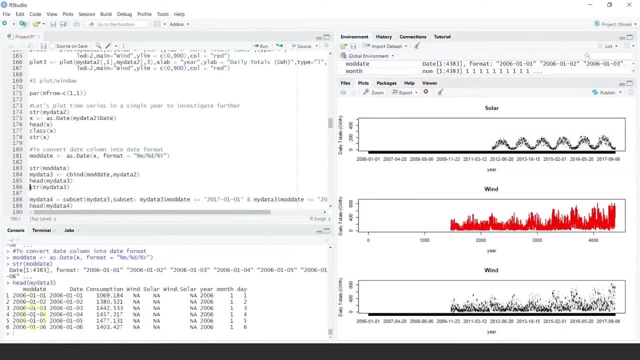 and then I can look at the head of it. so it says me mod data. now we are. what we did here is, when I said my data 3, so my data 3, we did a c bind and I did a mod data which is going to add this: 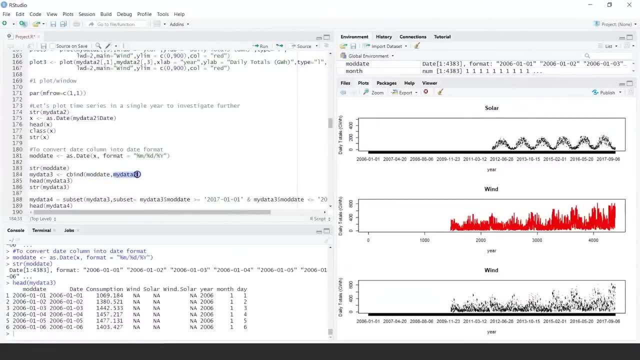 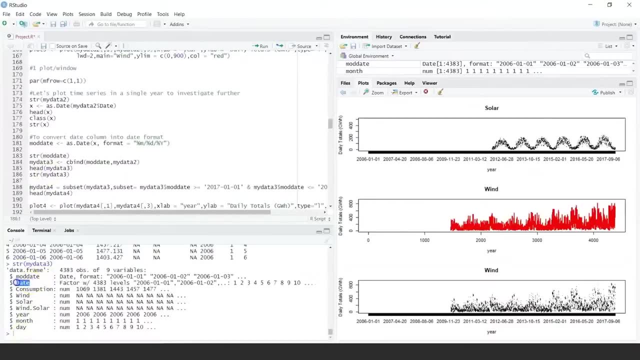 column to my other columns of my data 2. so my new data frame is my data 3. lets look at the structure of it and you see there is this date column. I can delete it. I can remove it, I can let it be right. so that depends on our choice. 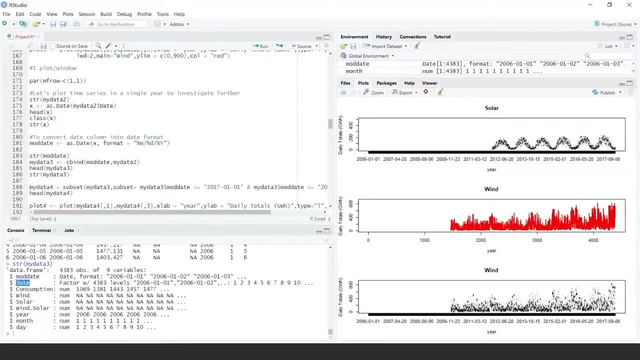 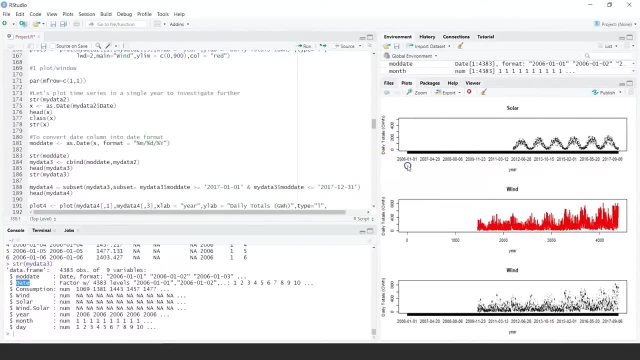 might be. we want to. once our analysis done, we want to remove the mod data right, so we can keep both of them. now lets basically extract data for a particular year. now, how do you do that? so this is some wrangling, so I will say my data. 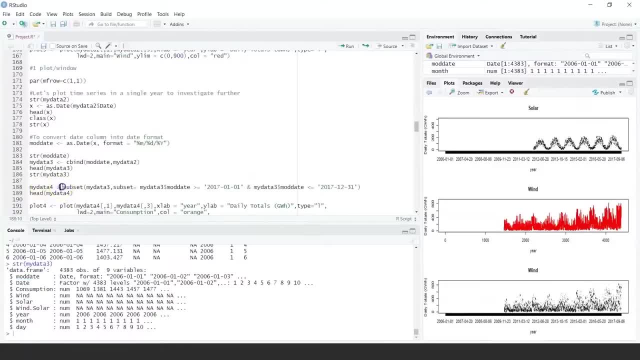 4, lets call it my data 4- and I will use subset function. so subset will work on my data 3. thats the data and what I will do is I will do a subset. how do how is the subset found? so I will say: take the mod data. 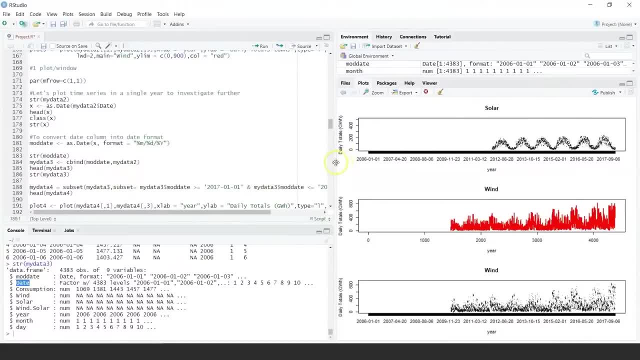 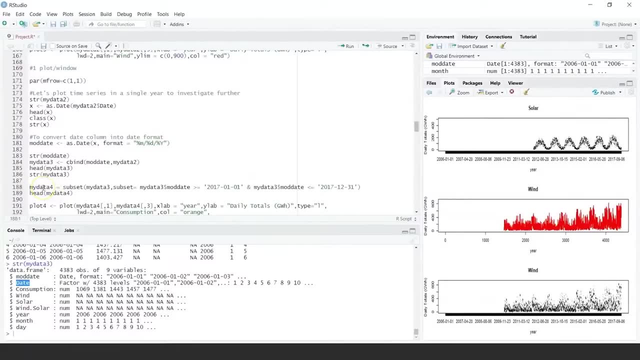 now let's basically extract data for a particular year. now how do you do that? so this is some wrangling. so i will say my data 4, let's call it my data 4, and i will use subset function. so subset will work on my data 3. that's the data. 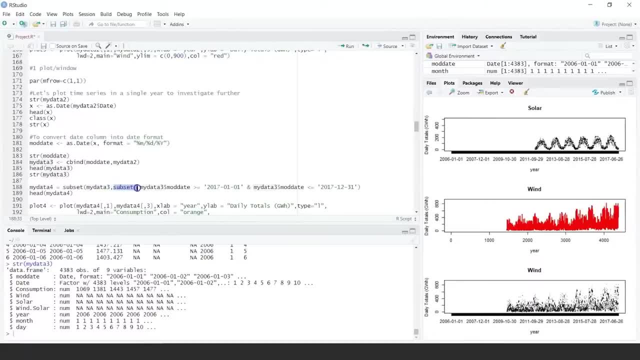 and what i will do is: i will do a subset. how do how is the subset found? so i will say, take the mod data column. the value should be greater than or equal to 2017 and should be less than 2017, December 31st. so i am. 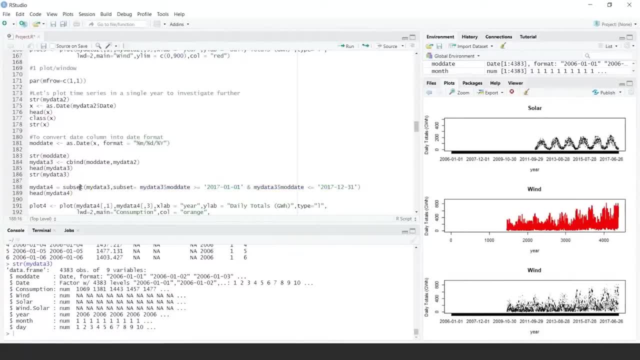 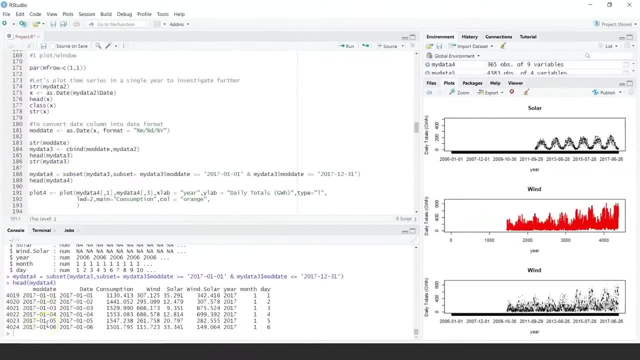 getting data for one year and i am storing it as my data 4. let's get the head of it and you see we are specifically looking at 2017 related data. now let's do a plotting of this, where i will only create a plot for one. 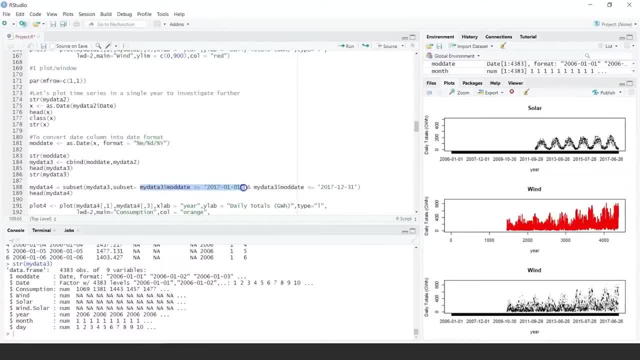 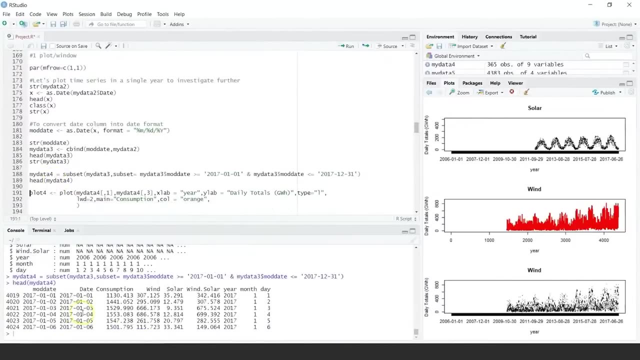 column. the value should be greater than or equal to 2017 and should be less than 2017 December 31st. so I am getting data for one year and I am storing it as my data. 4. lets get the head of it and you see. 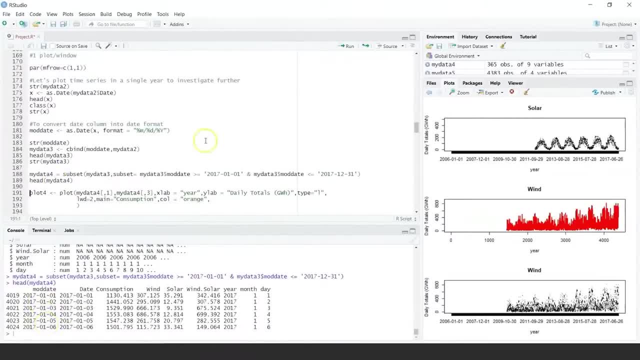 we are specifically looking at 2017 related data. now lets do a plotting of this, where I will only create a plot for one year. so I am saying my data 4, thats my new data, what we got. so here I am going to take the first column. 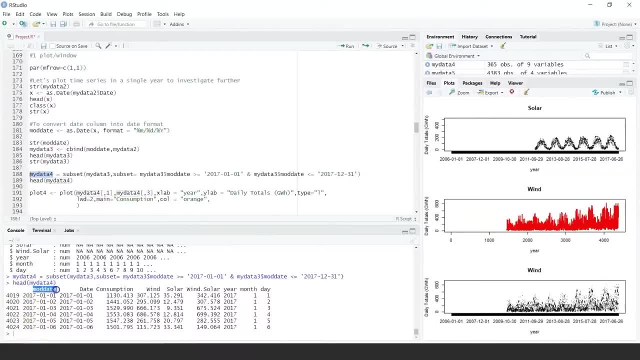 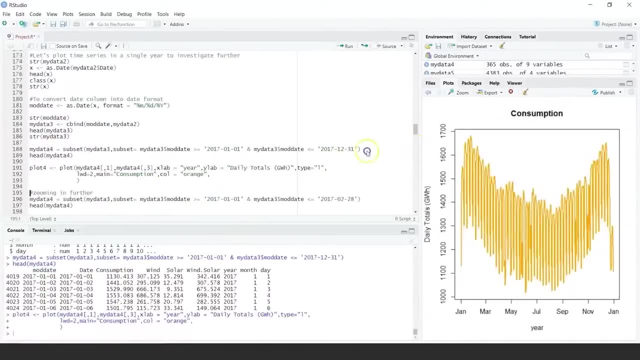 which is mod data. I am going to take the third column, which is consumption. so I am looking at the date format for one year, consumption values for it and then rest of the things. as we have done earlier, lets look at the plot, and this makes more meaning. 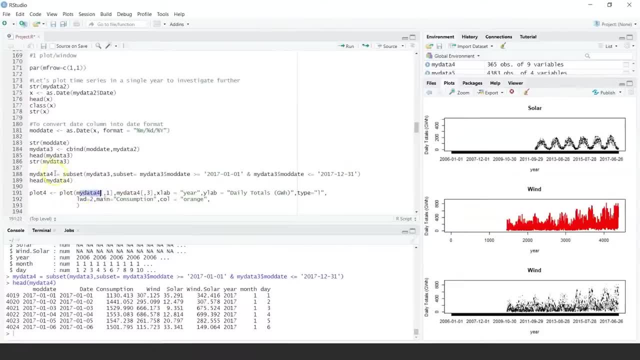 year. so i am saying my data 4, that's my new data, what we got. so here i am going to take the first column, which is mod data. i am going to take the third column, which is consumption. so i am looking at the date format for one year. 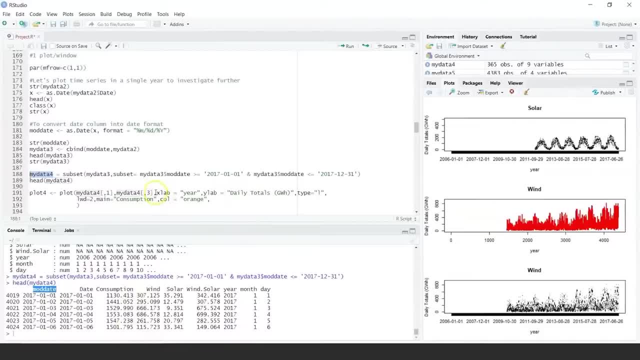 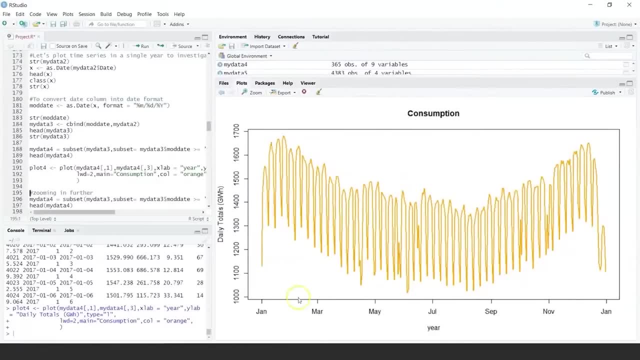 consumption values for it and then rest of the things. as we have done earlier, let's look at the plot, and this makes more meaning, right? so when you look at this plot, it tells me jan to jan. it shows me some kind of pattern where i have divided. 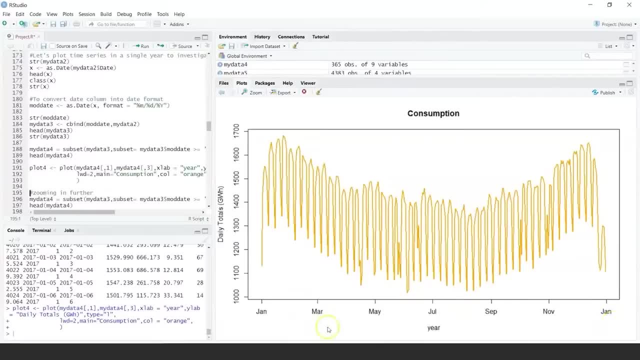 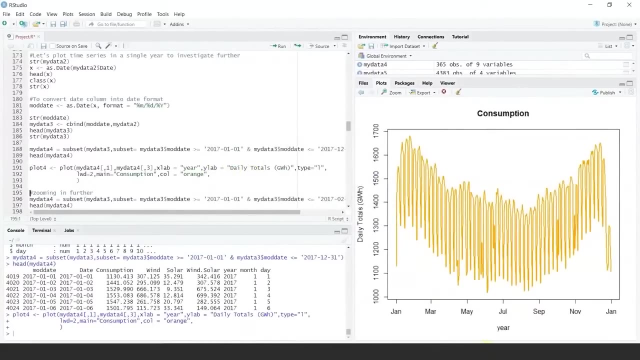 the year into months, right, and it is broken down into, say, two months, jan and march, and may and july and so on. but we still see a pattern- and that gives me good understanding of pattern- where i have broken it down into months. so this is where you have taken. 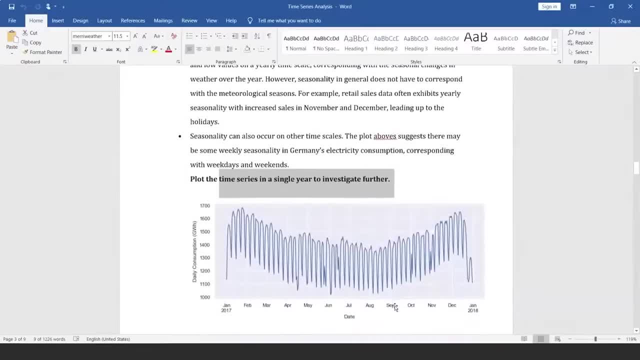 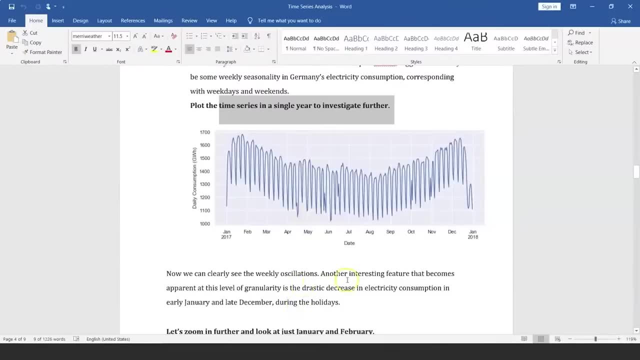 time series in a single year to investigate further. and this is what we see right now. we can clearly see there are some weekly oscillations. what one more interesting feature is that at this level of granularity- that is, when you are looking at yearly data- there is a drastic decrease. 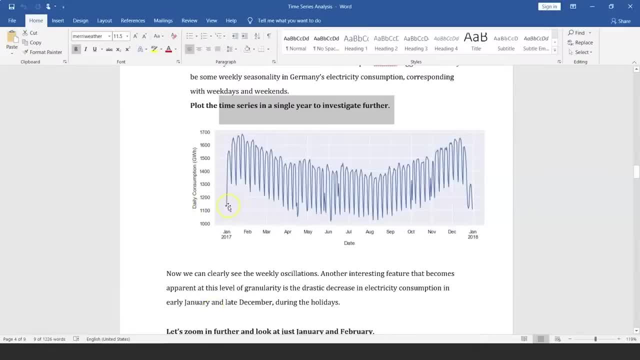 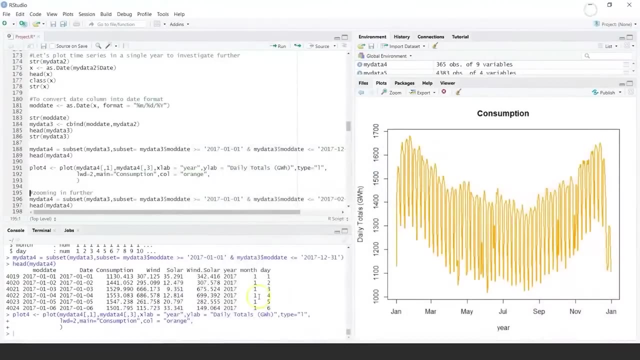 in electricity consumption in early january and late december during the holidays, or probably we can assume that this is holidays. now i can zoom in further and look at just jan and feb data. let's see how we do that and let's see how we work by zooming. 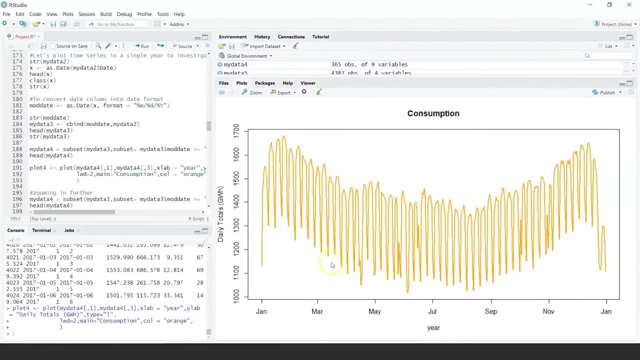 right. so when you look at this plot, it tells me jan to jan, it shows me some kind of pattern where I have divided the year into months, right, and it is broken down into, say, two months, so jan and march and may and july and so on. but we still see. 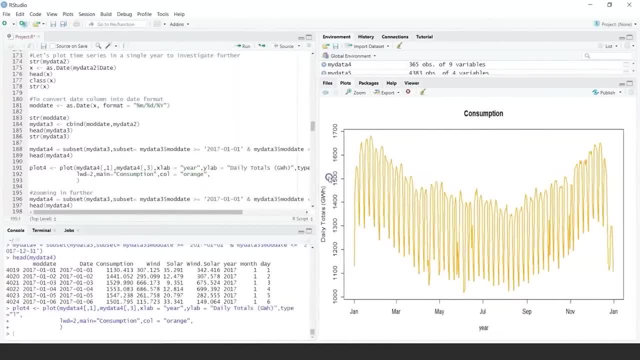 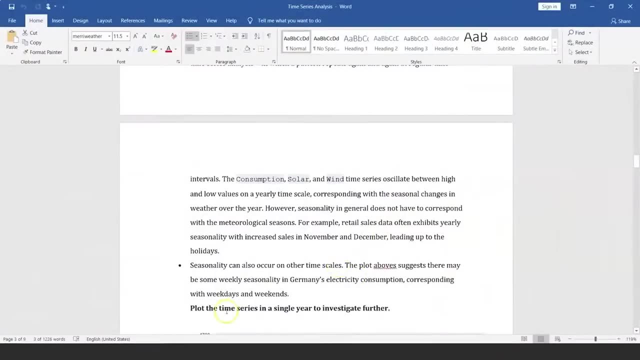 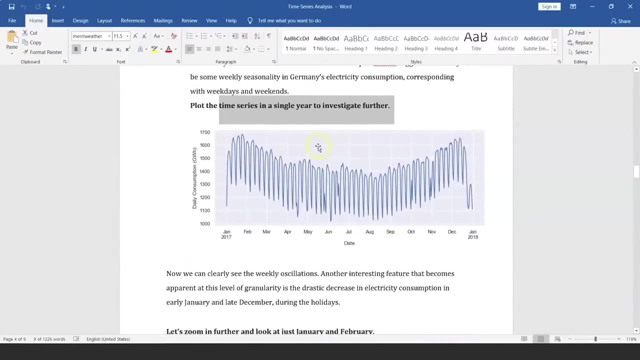 a pattern- and that gives me good understanding of pattern- where I have broken it down into months. so this is where you have taken time series in a single year to investigate further, and this is what we see right now. we can clearly see there are some weekly oscillations. what? 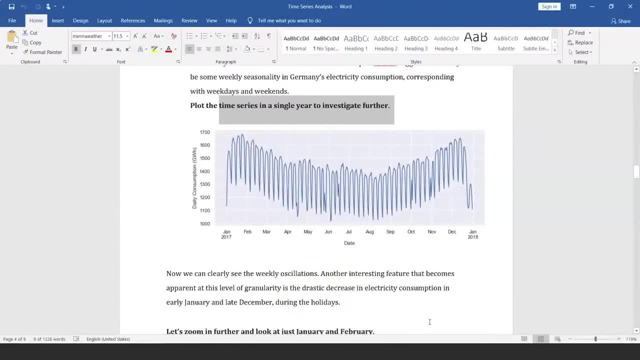 one more interesting feature is that at this level of granularity- that is, when you are looking at yearly data- there is a drastic decrease in electricity consumption in early january and late december, during the holidays, so probably we can assume that this is holidays. now I can zoom in further. 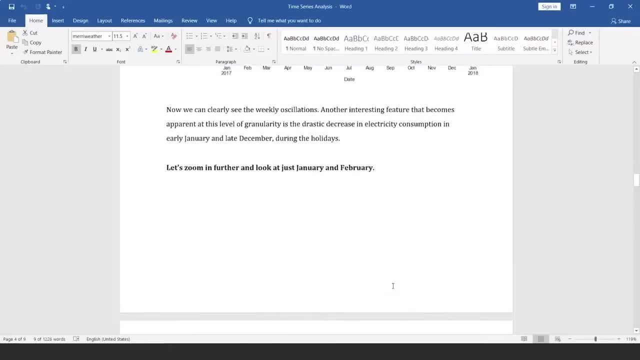 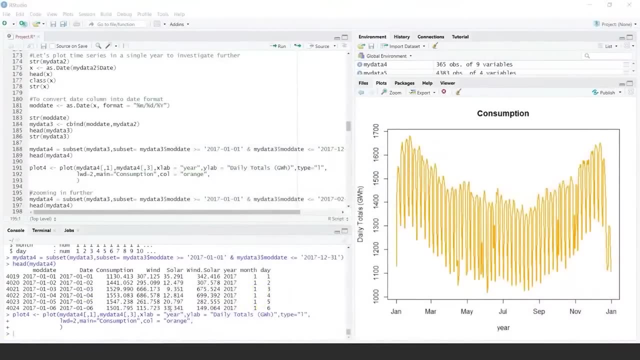 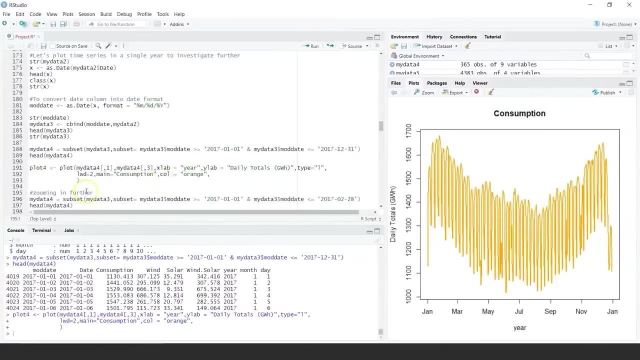 and look at just jan and feb data. lets see how we do that and lets see how we work by zooming in the data further. so, to zoom in the data further, lets see how we do it. now, here we have this, my data 4, which is basically having a subset. 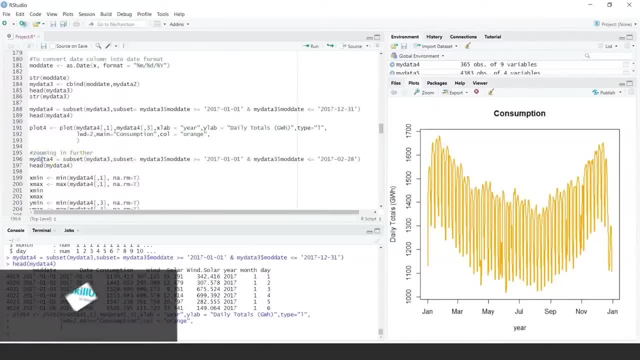 right, so lets work on this one. so I will say my data 4, which earlier I was taking data 3. I was doing a subset and I was giving the date, but this time I will make it more narrower, so I will say my data 4. 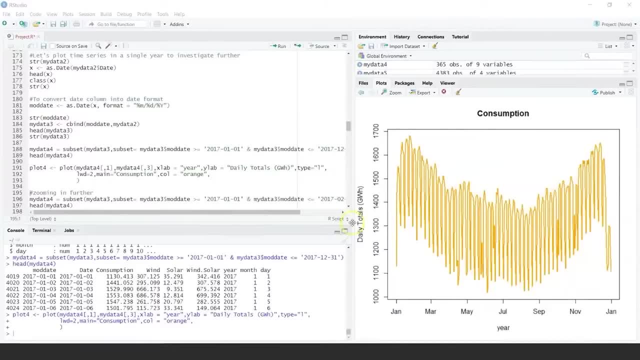 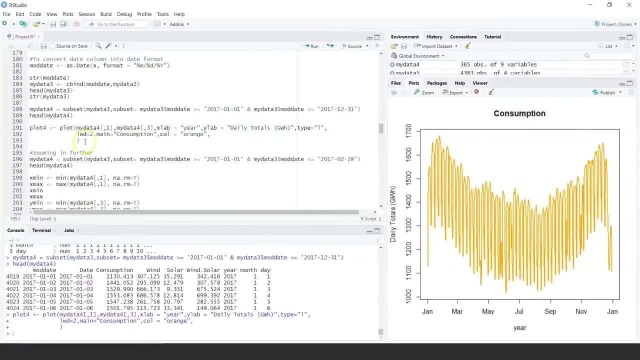 in the data further. so, to zoom in the data further, let's see how we do it. now, here we have this, my data 4, which is basically having a subset right. so let's work on this one. so i will say my data 4, which earlier i was taking. 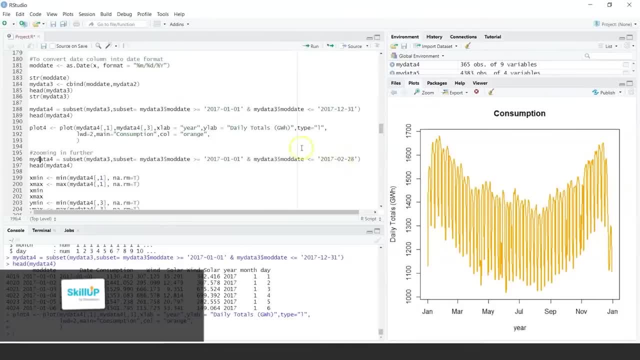 data 3. i was doing a subset and i was giving the date, but this time i will make it more narrower, so i will say my data 4, i will say subset from my data 3 and i will choose mod data column, which we have modified with the date format. 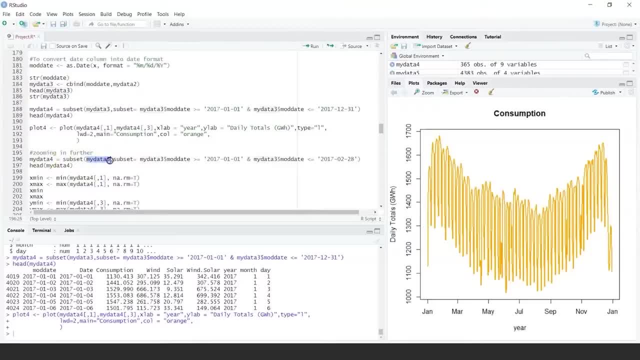 I will say subset from my data 3 and I will choose mod data column, which we have modified with the date format. I will choose the starting date as 1701, that is, jan, and then lets go till feb and lets create this. now lets look at the head. 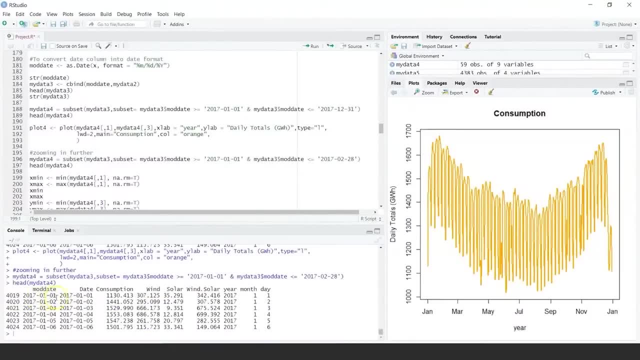 of this. so it shows me we have the data, which is jan, and then you can basically look at more on this. now again, as I said earlier, lets find out the minimum of this from the first column. so that is basically your mod data. so lets look into this one and that. 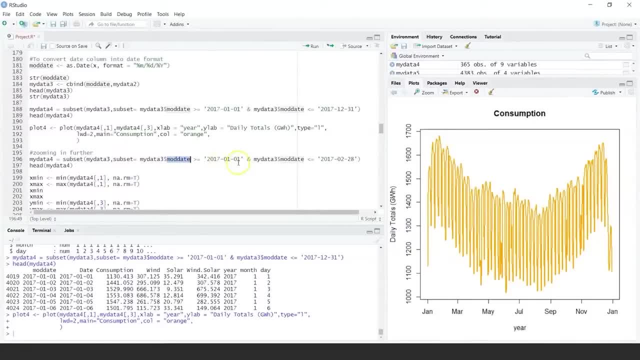 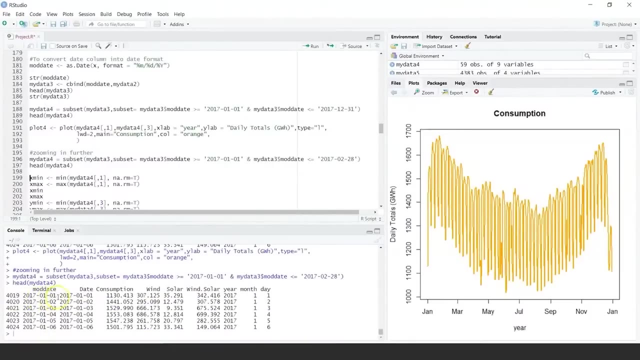 i will choose the starting date as 1701, that is, jan, and then let's go till feb and let's create this. now. let's look at the head of this so it shows me we have the data, which is jan, and then you can basically look at more. 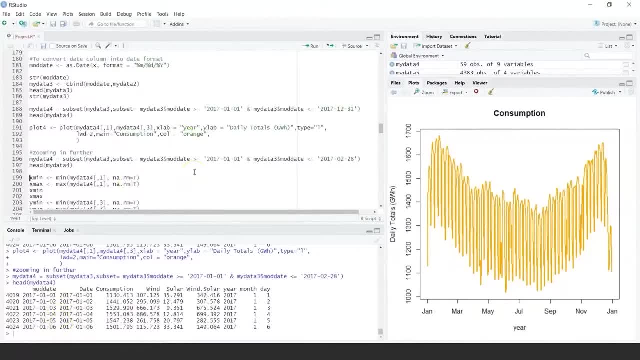 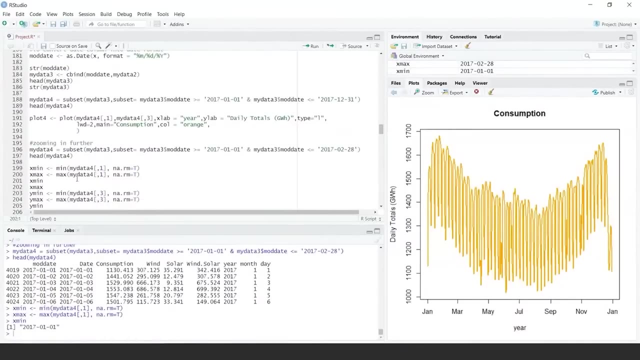 on this now again, as i said earlier, let's find out the minimum of this from the first column. so that is basically your mod data. so let's look into this one and that basically will give me minimum and maximum. let's look at the values. so this: 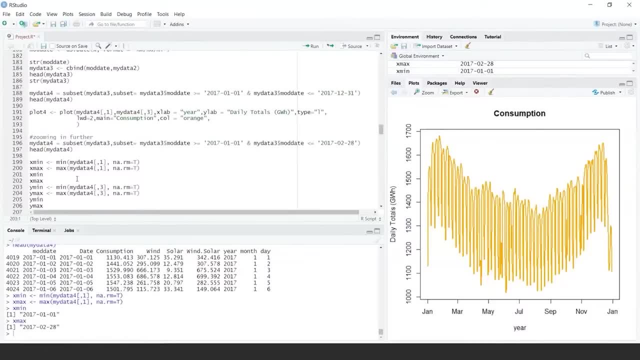 one tells me jan 17, january 1 and maximum is your feb 28, second month 2017. so we are actually looking at 2 months data here. let's look at the y minimum. so this is. i will look at column 3 now. what is column 3? 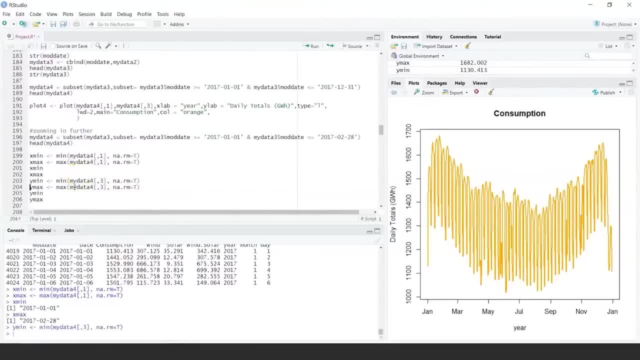 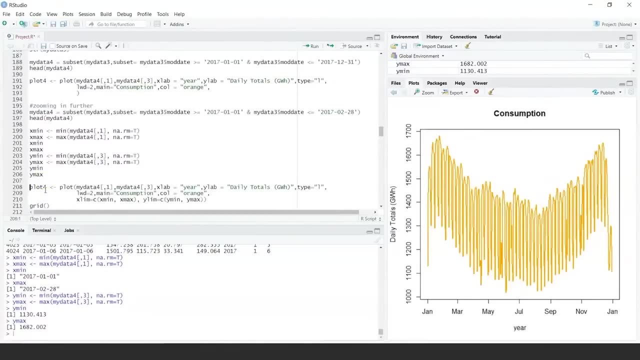 consumption. so let's look at the minimum value for consumption, maximum value of consumption. let's look at the values which can be given as our limits. now, this is the minimum and maximum. now let's do a plotting for this data, which has been narrowed down for consumption, based on my data. so 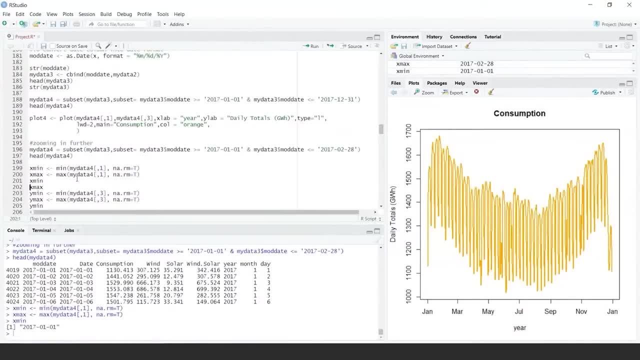 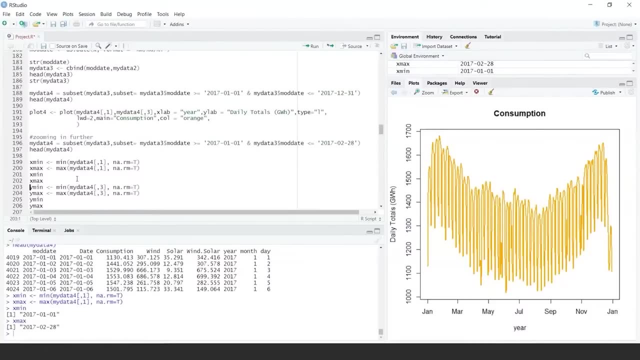 basically will give me minimum and maximum. lets look at the values. so this one tells me jan 17, january 1 and maximum is your feb 28, second month 2017. so we are actually looking at 2 months data here. lets look at the y minimum. 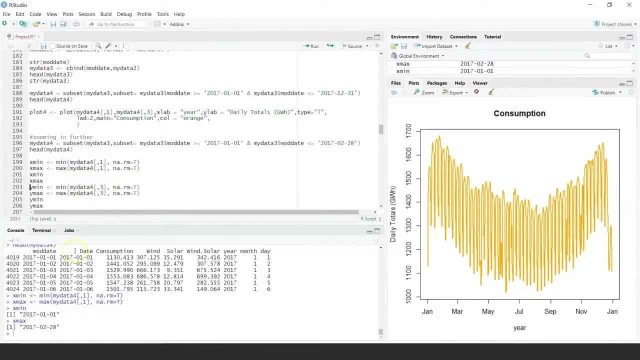 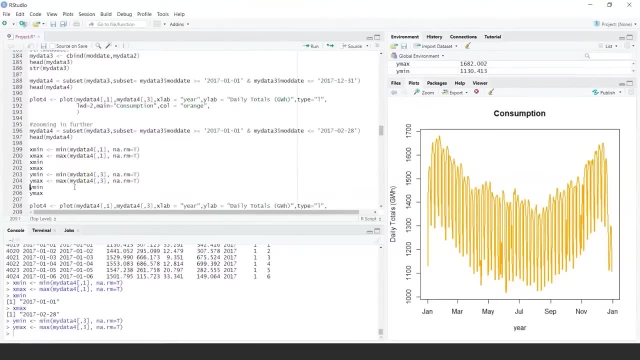 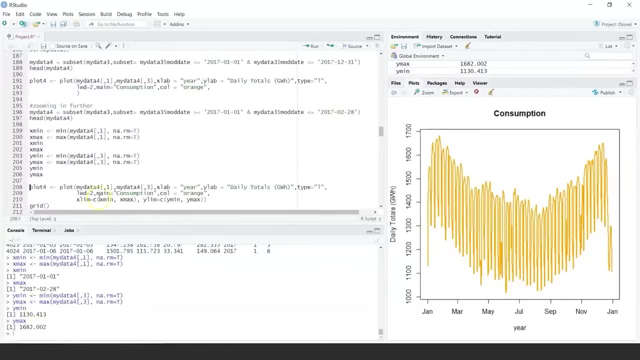 so this is. I will look at column 3 now. what is column 3? consumption. so lets look at the minimum value for consumption, maximum value of consumption. lets look at the values which can be given as our limits. now, this is the minimum and maximum. now lets do a 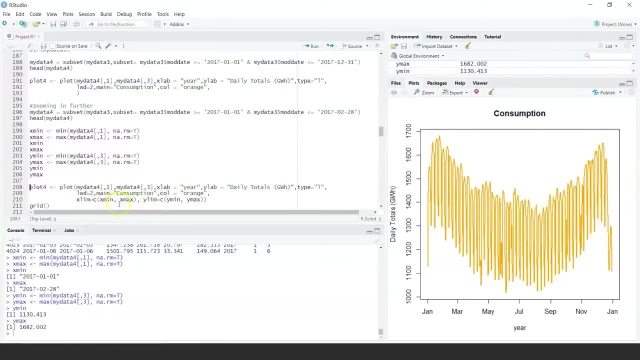 plotting for this data, which has been narrowed down for consumption based on my data. so I am saying my first column, which is mod data, and then third column, which is consumption. I am giving some naming convention for sorry naming for your x axis, y axis, what is my consumption? 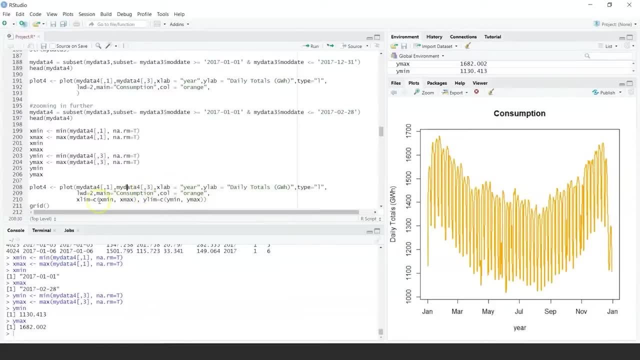 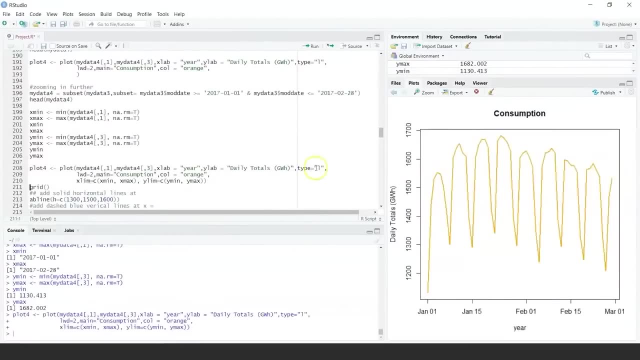 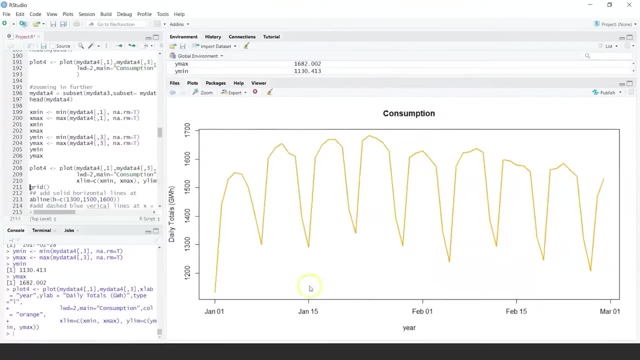 or what is my title here? what is the colour? and then you see I am using x limit to give the minimum and maximum limit and y limit. so lets look at this data. and if you look at this data it is specifically for 2 months. and again I can look at: 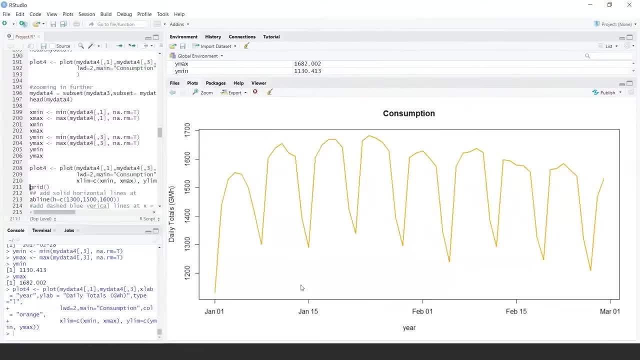 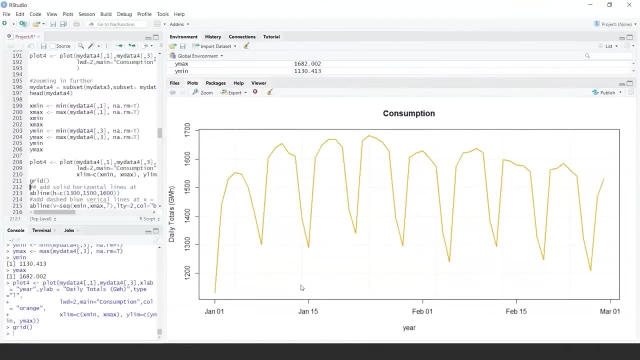 the pattern here. what I can also do is I can add some grid here so I can basically look at this data and make more meaning out of it. so it is bi weekly data. you can see now. I can add a line here using ab line and then I can basically choose. 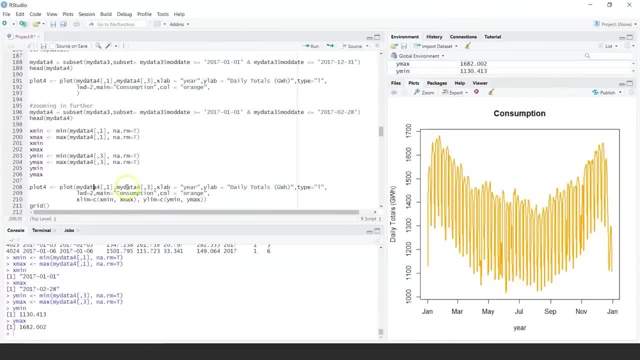 i am saying my first column, which is mod data, and then third column, which is consumption. i am giving some naming convention for sorry naming for your x axis, y axis, what is my consumption or what is my title here? what is the color? and then you see, i am using x limit. 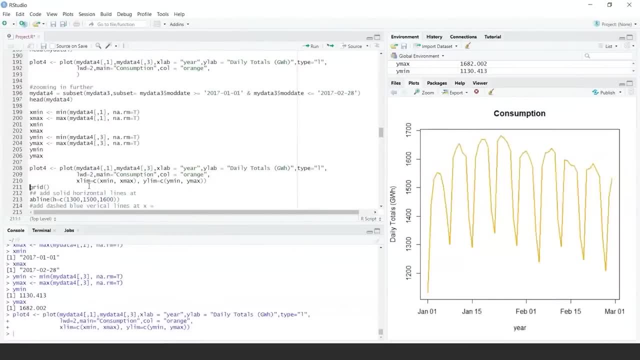 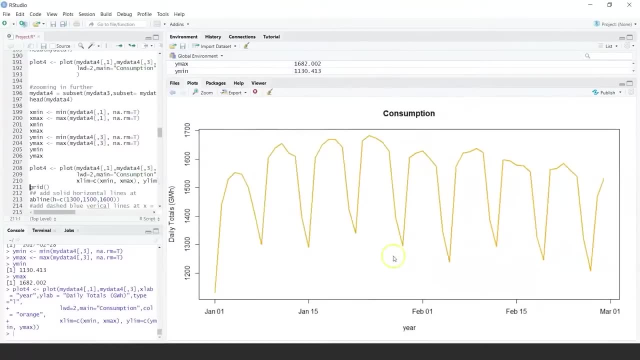 to give the minimum and maximum limit and y limit. so let's look at this data. and if you look at this data, it is specifically for 2 months and again i can look at the pattern here. what i can also do is i can add some grid here. 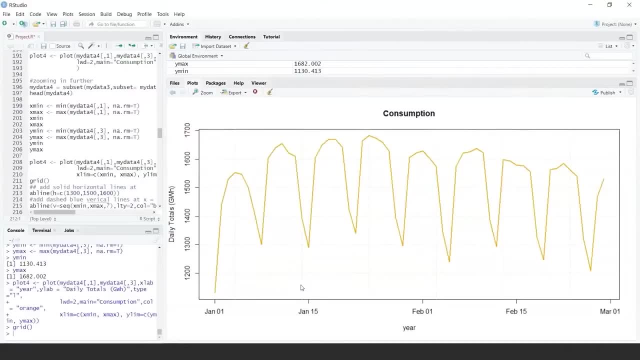 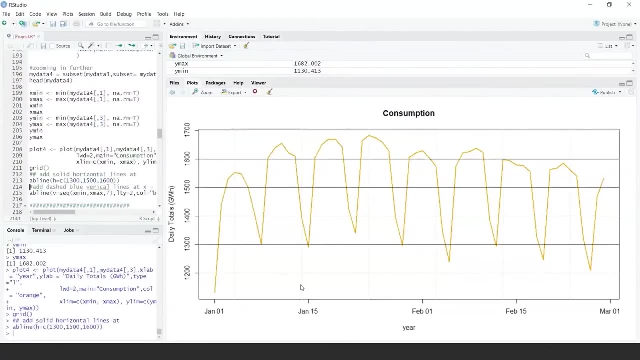 so i can basically look at this data and make more meaning out of it. so it is bi weekly data. you can see, now i can add a line here using ab line and then i can basically choose what lines i would want to add horizontally. so that basically allows me to dissect. 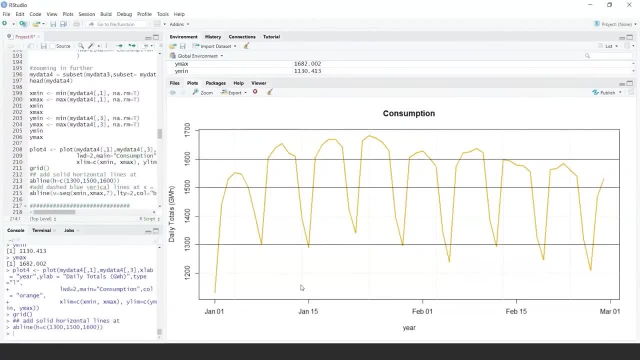 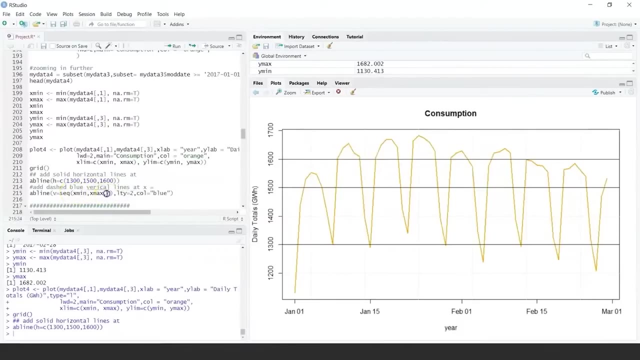 what lines I would want to add horizontally, so that basically allows me to dissect the data and look at data in a more meaningful way. I can also add vertical lines. so vertical lines is I am saying sequence will be minimum, maximum, and I am saying interval of 7. so lets. 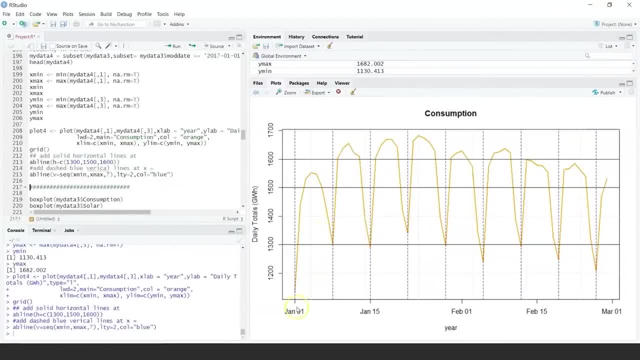 do this and this basically has added some lines every week and you can see at the end of week it is dropping and then it is starting again. it peaks somewhere in the mid of the week and again it drops down. so this is: you are looking at your consumption data. 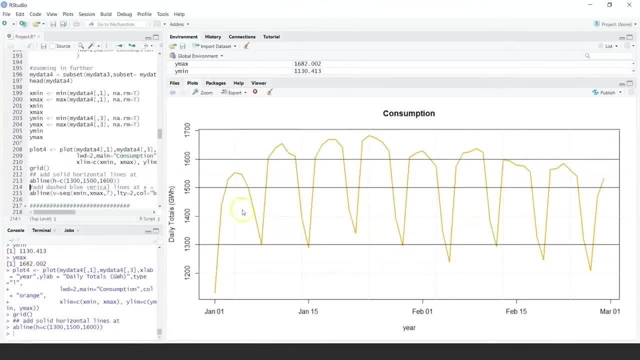 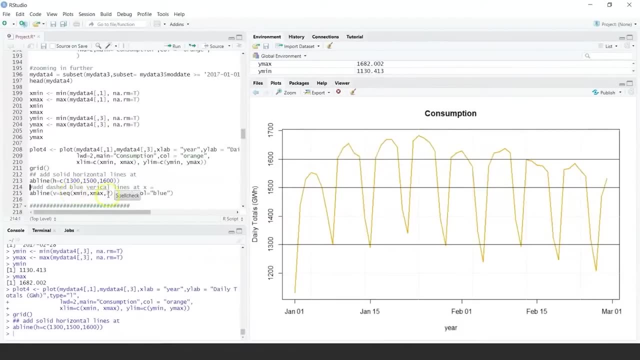 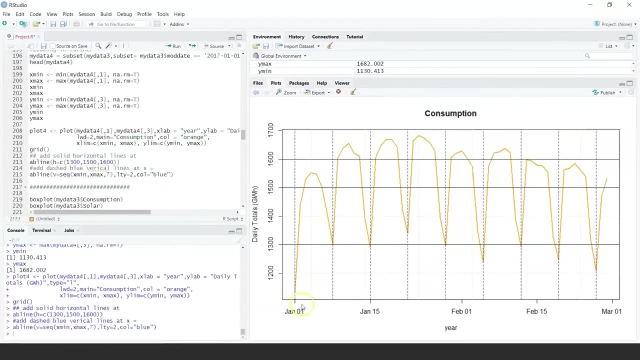 the data and look at data in a more meaningful way. i can also add vertical lines. so vertical lines is i am saying sequence will be minimum, maximum and i am saying an interval of 7, so let's do this, and this basically has added some lines every week and you can see. 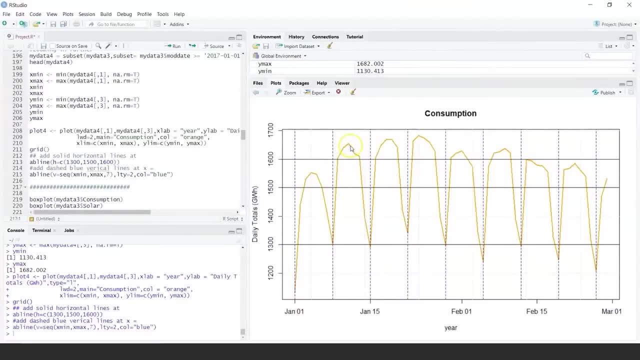 at the end of week it is dropping and then it is starting again. it peaks somewhere in the mid of the week and again it drops down. so this is: you are looking at your consumption data. now. what we can also do is we can create some box plots. so 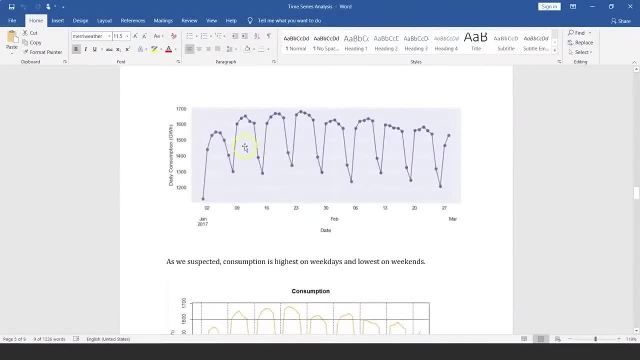 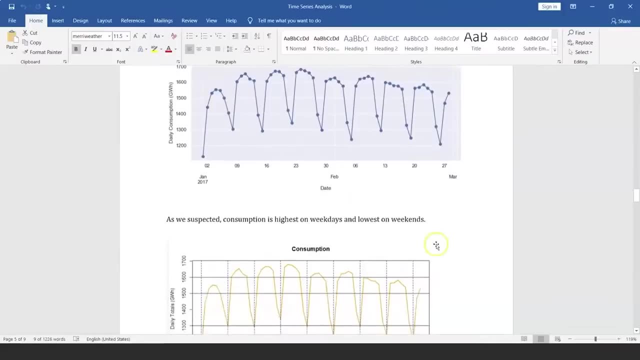 when we looked at zooming in data for jan and feb, you can add some data points like this: so consumption is highest on the week days, as i showed you here, and lowest on the weekends. so this is what we are seeing when we are breaking the data or zooming it. 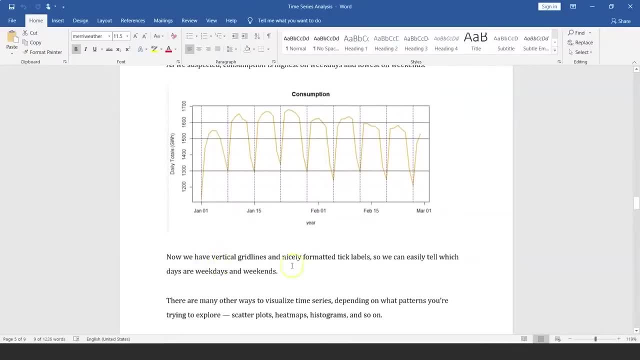 further for couple of months. so we have vertical grid lines and we have nicely formatted tick labels that is jan first, jan 15 feb first, and so on. so we can easily tell which days are week days and weekends with use of these grid lines and basically breaking it down. 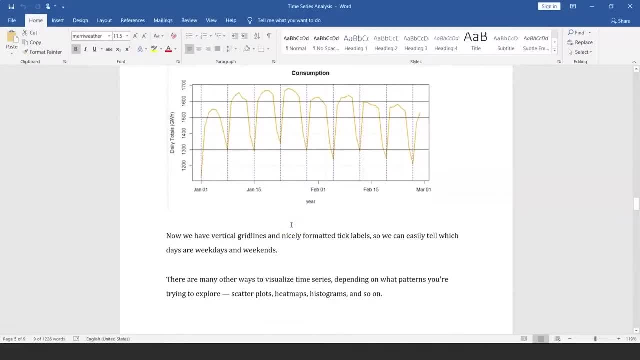 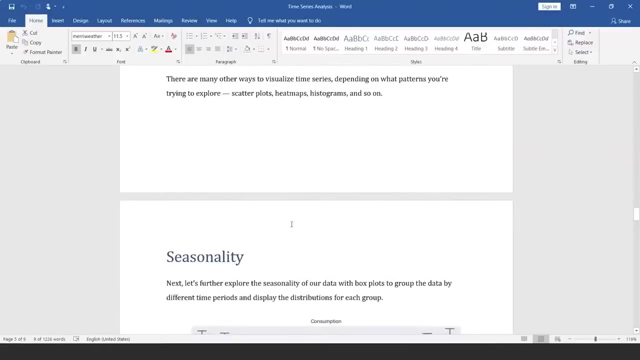 so there are many other ways to actually visualize your time series data, depending on what patterns you are trying to explore. you can use scatter plots, you can use heat maps, you can use histograms, and so on. now, moving further, we would want to explore the seasonality right. so when you 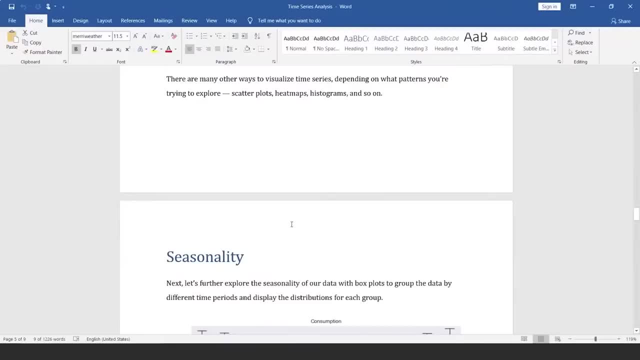 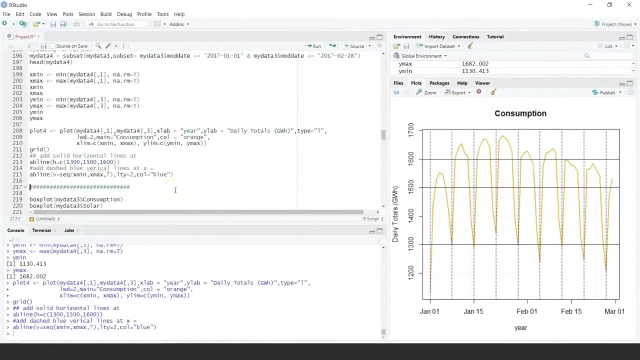 further explore the seasonality of our data. we can use box plots basically to group the data by different time periods and display the distribution for each group. now how do we do that? lets come here and lets see how box plot works. so i can just do a simple box plot. 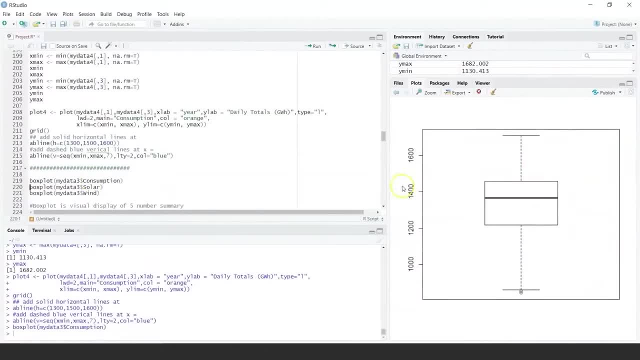 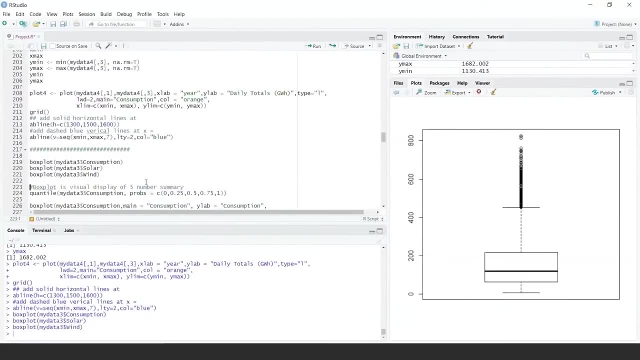 and i can choose my consumption column and that gives me just the consumption data. but this really does not give me any meaning. i can look at solar data, i can look at the wind data and we can also see some outliers here, so we can create box plots. but if we 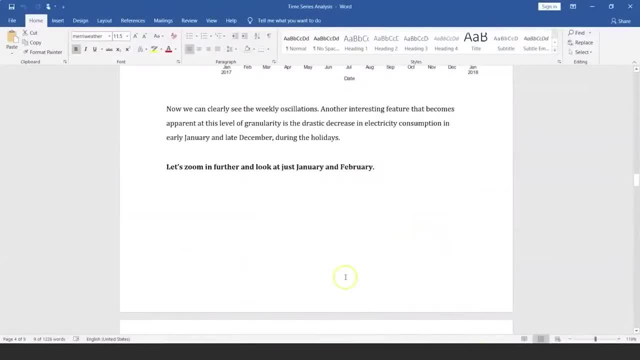 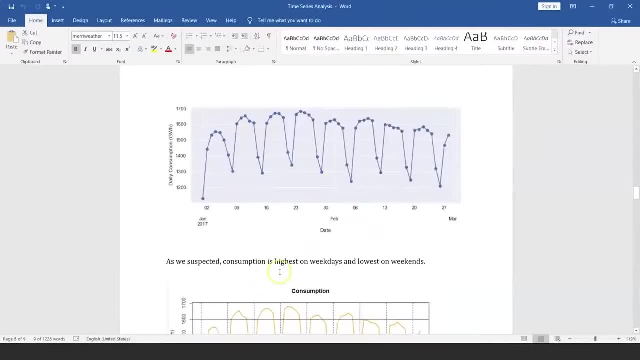 right now. what we can also do is we can create some box plots. so when we looked at zooming in data for Jan and Feb, you can add some data points like this: so consumption is highest on the weekdays, as I showed you here, and lowest on the weekends. 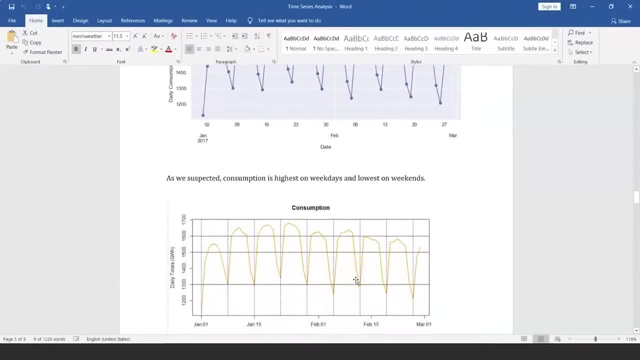 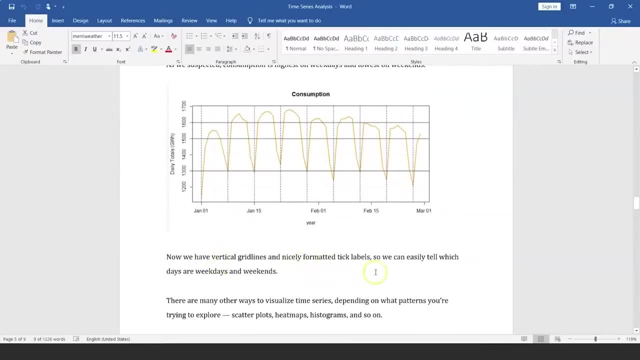 so this is what we are seeing when we are breaking the data or zooming it further for couple of months. so we have vertical grid lines and we have nicely formatted tick labels. that is Jan 1st, Jan 15th, Feb 1st and so on, so we can. 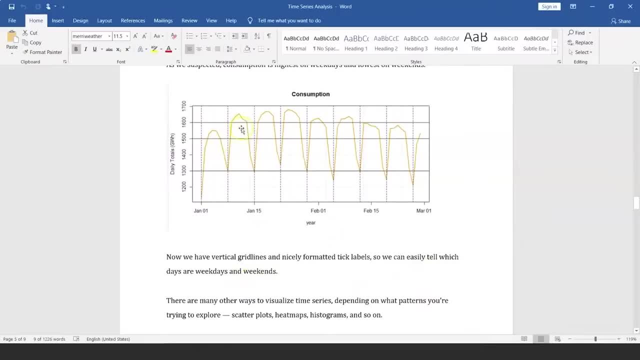 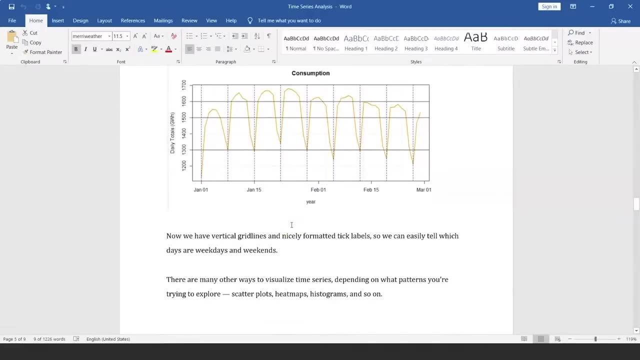 easily tell which days are weekdays and weekends with use of these grid lines and basically breaking it down. so there are many other ways to actually visualize your time series data, depending on what patterns you are trying to explore. you can use scatter plots, you can use heat maps, you can 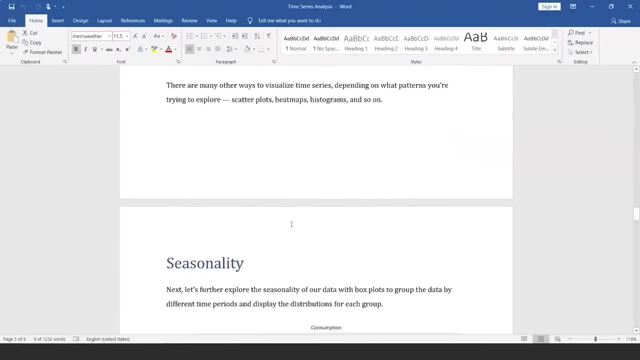 use histograms and so on. now, moving further, we would want to explore the seasonality right? so when you further explore the seasonality of our data, we can use box plots basically to group the data by different time periods and display the distribution for each group. now, how do we do that? 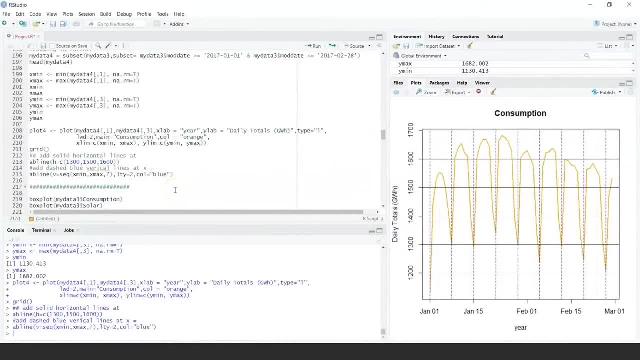 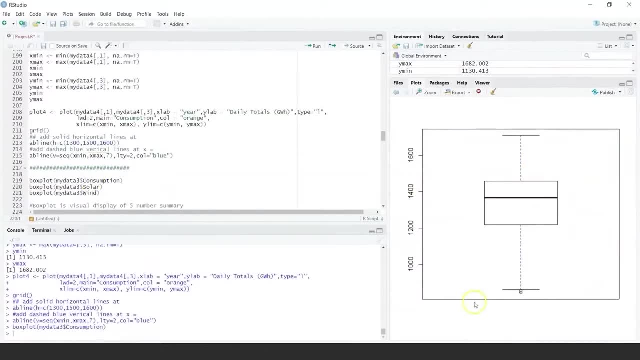 let's come here and let's see how box plot works. so I can just do a simple box plot and I can choose my consumption column and that gives me just the consumption data. but this really does not give me any meaning. I can look at solar data. 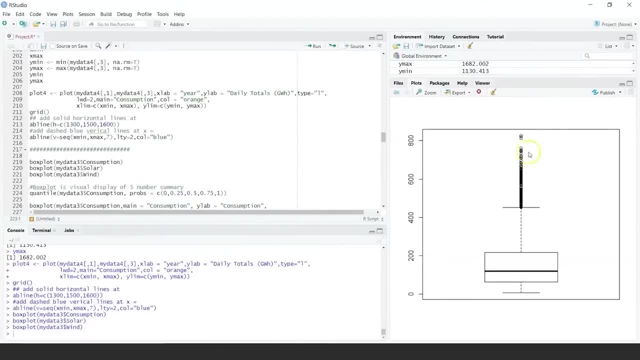 I can look at the wind data and we can also see some outliers here so we can create box plots. but if we would want to do a box plot, what is box plot? it is basically a visual display of your phi number summary, that is, you want to. 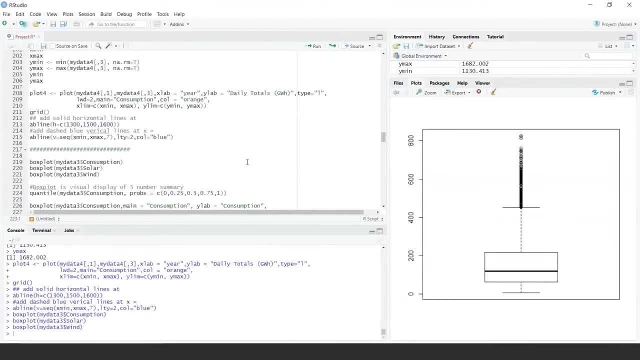 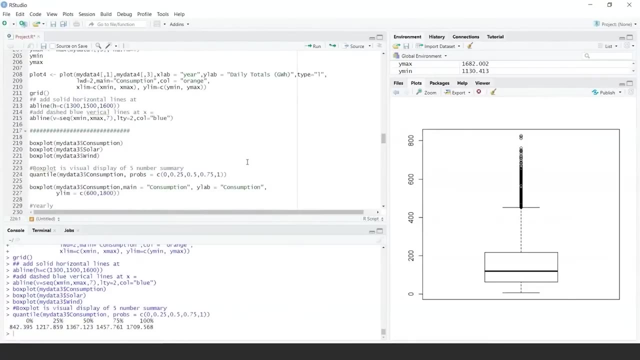 look at your mean median. you want to look at your 25th percentile, 50th percentile or 75th percentile. so we can use a quantile function, use the consumption column and then you basically give a vector which shows you phi number summary. so that's. 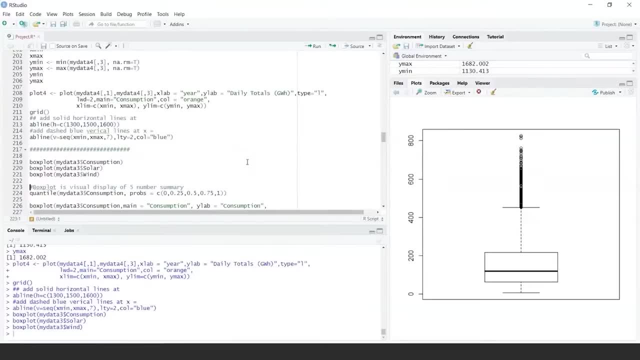 would want to do a box plot. what is box plot? it is basically visual display of your phi number summary. that is, you want to look at your mean median, you want to look at your 25th percentile, 50th percentile or 75th percentile, so we can use a quantile function. 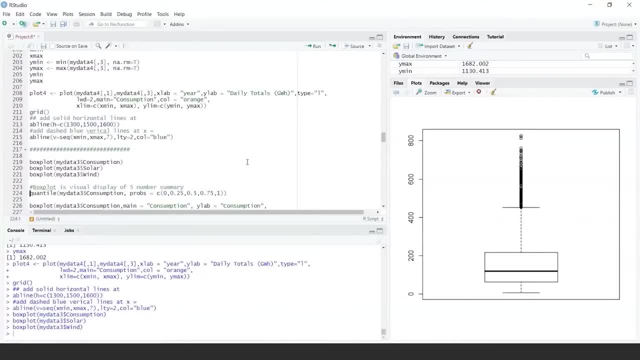 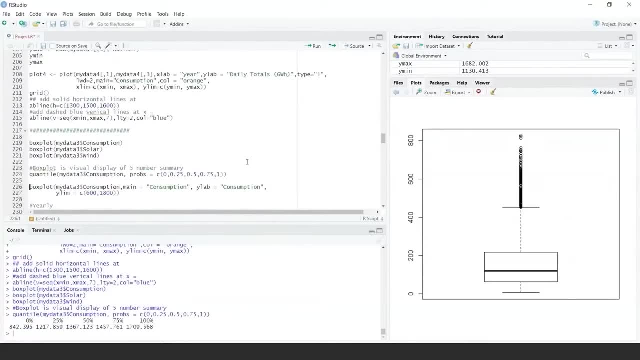 use the consumption column and then you basically give a vector which shows you phi number summary. so thats your quantile. and then lets do a box plot. so if you are looking at quantile, it tells me what is the minimum, what is 25th percentile 50. 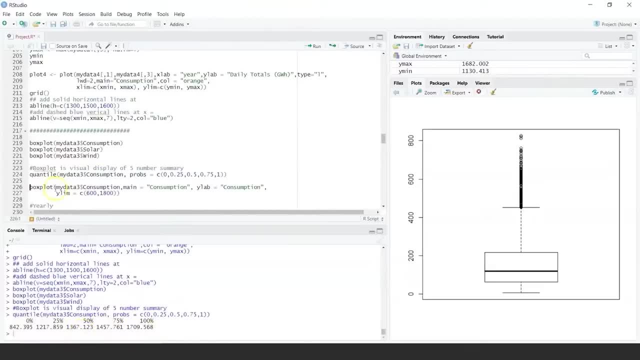 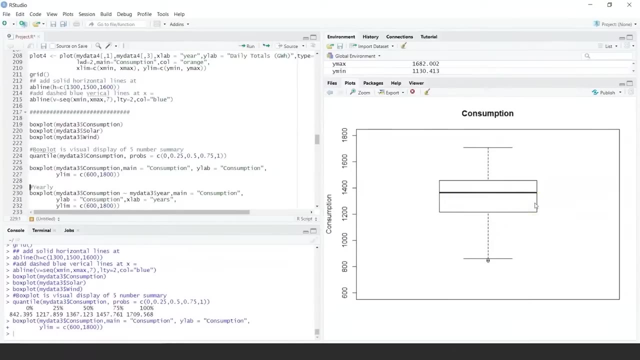 75th and 100. thats from my consumption column. so lets create a box plot for consumption. lets give it a name as consumption. lets give y axis as consumption and a limit for y axis. now thats my consumption graph. so i can look at yearly data now. that will make more meaning. 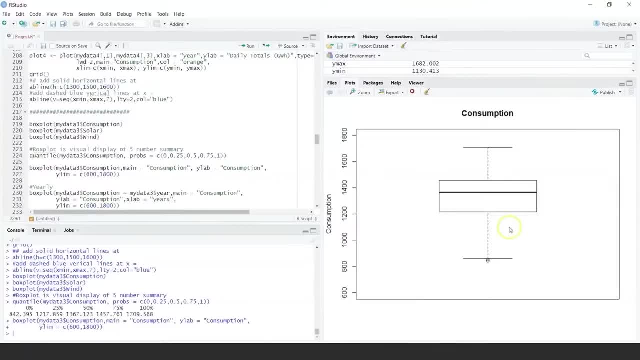 rather than just looking at the complete consumption data. so how do we do it? yearly? so we will say consumption and then i will say the year column. so it is consumption, but grouped based on year. so here i can give x axis, y axis and i can give y limit. 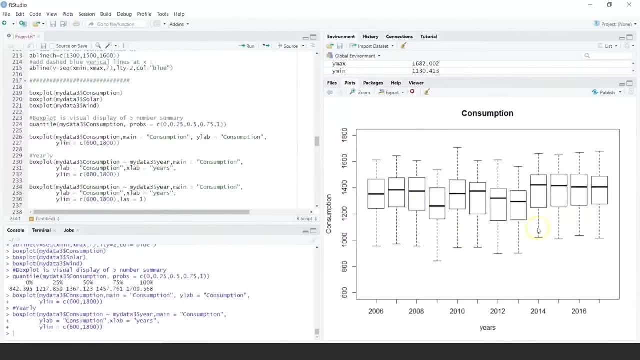 so lets create this, and this makes more meaning. we can give some coloring scheme here. but now i am looking at 2006, 2007, 8, 9 and so on, and we can look at the data. what is the range? right? it gives me 5 percentile, or, sorry, 5. 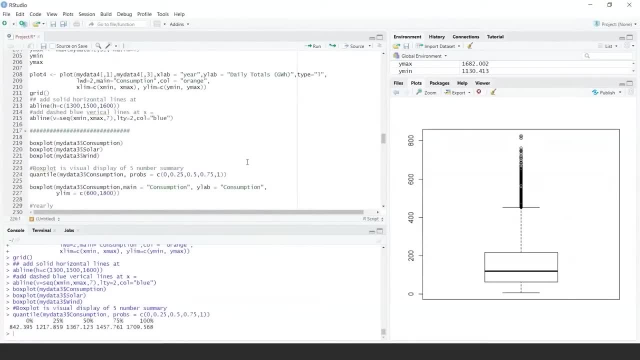 your quantile and then let's do a box plot. so if you are looking at quantile, it tells me what is the minimum, what is 25th percentile, 50th, 75th and 100th. that's from my consumption column. so let's. 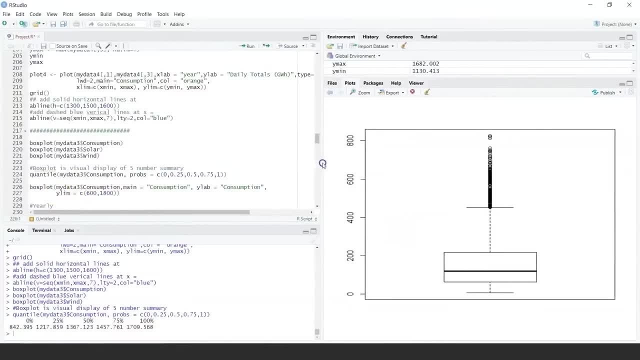 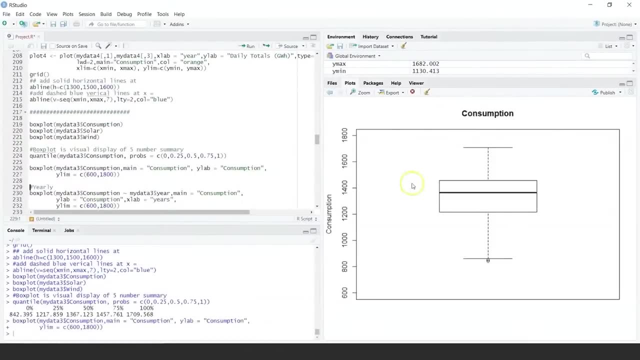 create a box plot for consumption. let's give it a name as consumption. let's give y axis as consumption and a limit for y axis. now that's my consumption graph, so I can look at yearly data now. that will make more meaning rather than just looking at. 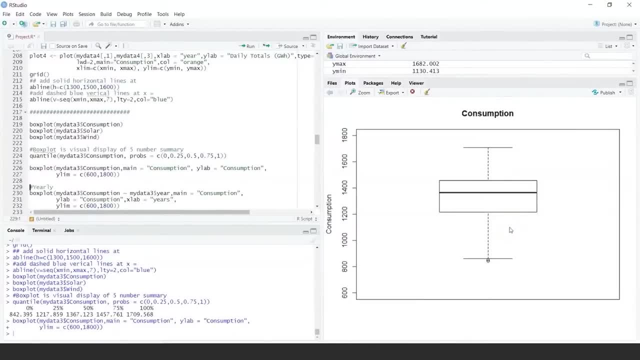 the complete consumption data. so how do we do it? yearly? so we will say consumption and then I will say the year column. so it is consumption, but grouped based on year. so here I can give x axis, y axis and I can give y limit. so let's create this. 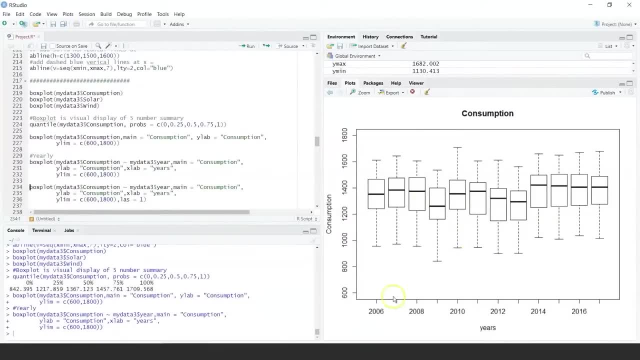 and this makes more meaning. we can give some coloring scheme here, but now I am looking at 2006, 2007, 8, 9 and so on and we can look at the data. what is the range? right? it gives me 5 percentile, or sorry. 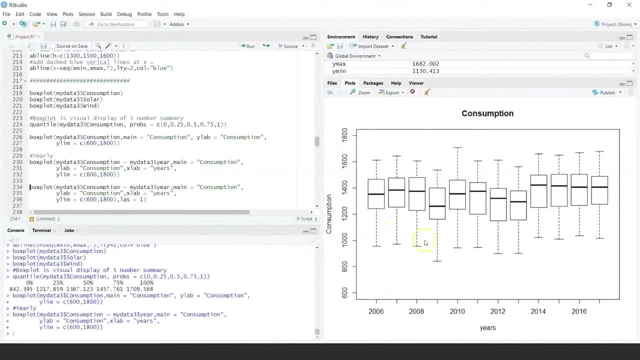 5 number summary of the data per year and it basically allows me to look at the seasonality of this. similarly, we can create box plot by just giving consumption yearly grouped, and here I am giving the title as consumption y axis, x axis and y limit, where in I can also use 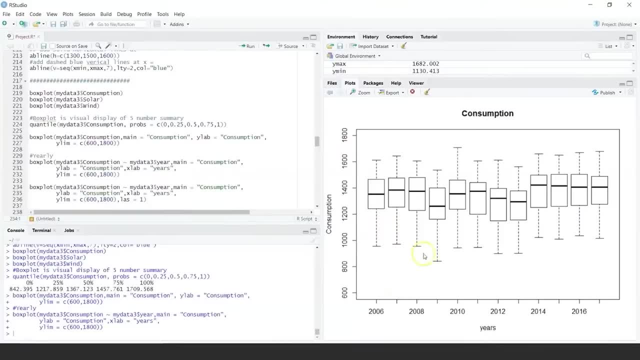 number summary of the data per year, and it basically allows me to look at the seasonality of this. similarly, we can create box plot by just giving consumption yearly grouped, and here i am giving the title as consumption y axis, x axis and y limit, where in i can also use less. 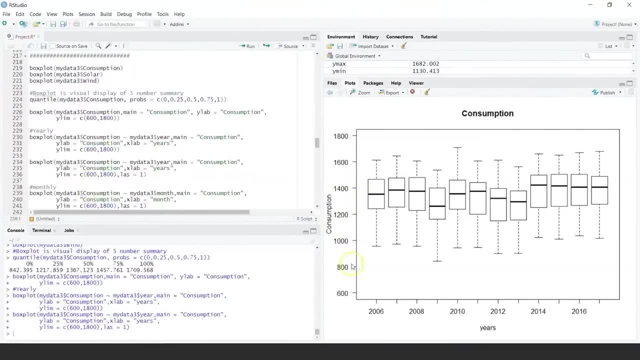 so this is one more feature which you can do and that basically will give me the tick points if you compare this one to the previous graph. so when i created this previous graph, i had 2006, 2008 and i had from 1600 to 1800, and if 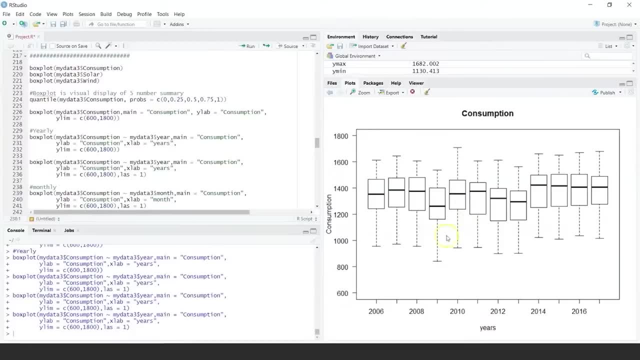 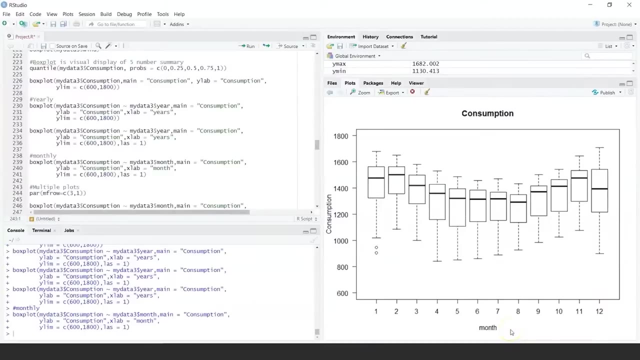 i go for the next one. i am basically seeing more useful information now. lets look at monthly data, so i would want to group it based on months and lets create that. so this gives me the monthly data, where i am looking at months and i could select a. 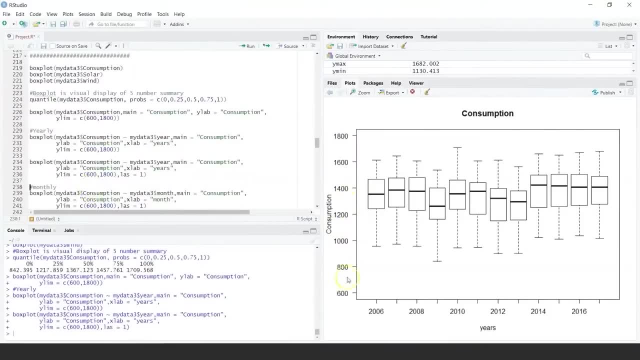 less. so this is one more feature which you can do and that basically will give me the tick point if you compare this one to the previous graph. so when I created this previous graph, I had 2006, 2008 and I had from 600 to 1800. 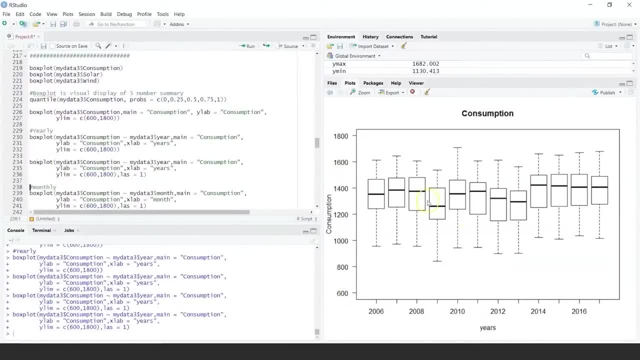 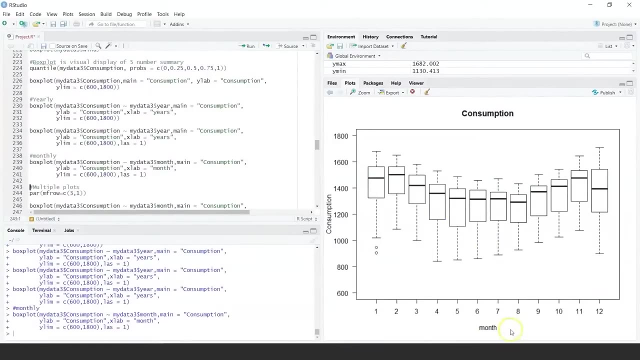 and if I go for the next one, I am basically seeing more useful information. now let's look at monthly data, so I would want to group it based on months and let's create that. so this gives me the monthly data, where I am looking at months and I could select. 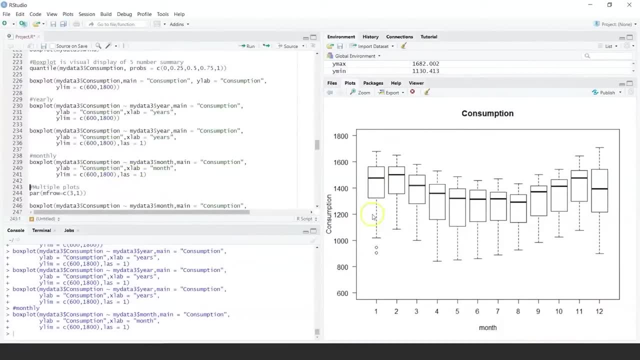 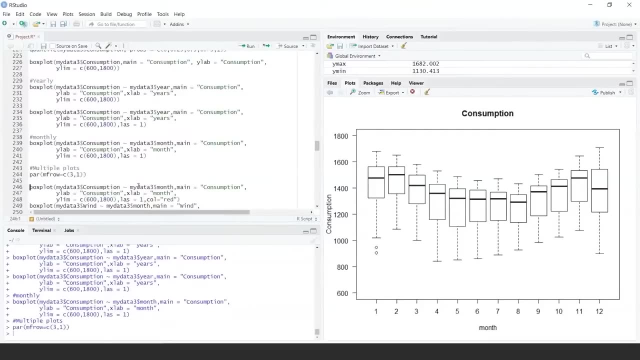 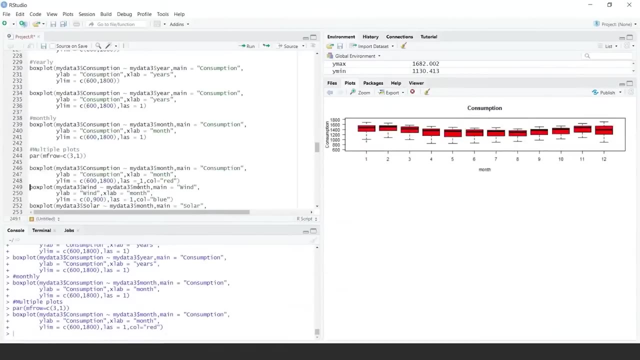 a particular year, or I can just do a grouping based on months so I can have multiple plots to see a difference here. so let's do this now. let's create a box plot for consumption, which is monthly data, and let's give it a color. let's look at the 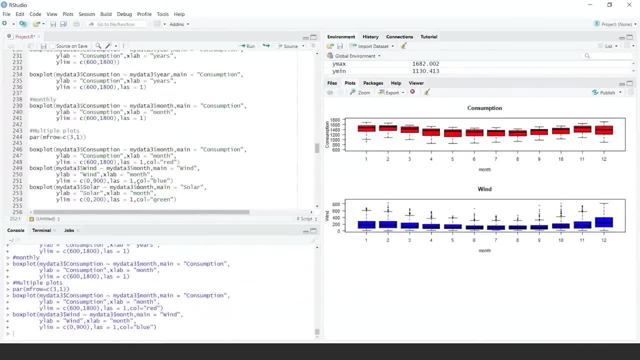 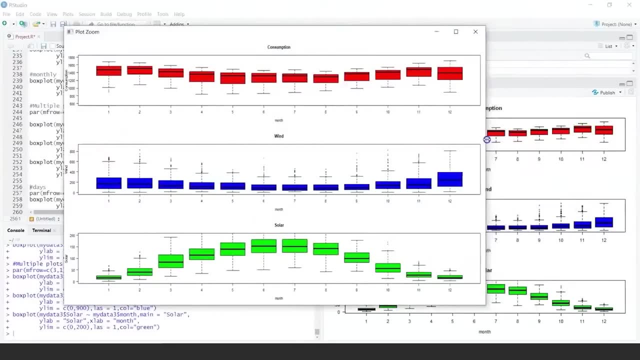 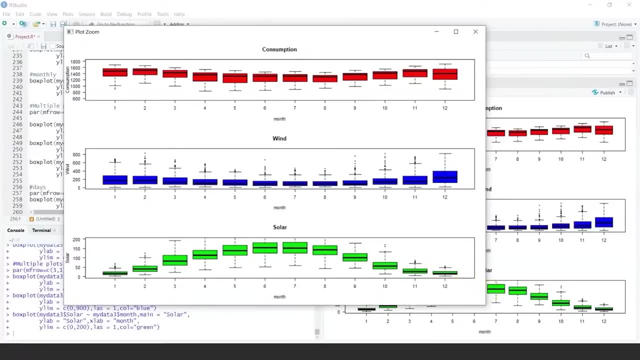 wind data, which is again grouped monthly. and let's look at the solar data, which is grouped monthly. now, if I zoom in, it basically gives me the seasonality of the data for your wind, for your consumption, for your solar. so what we are doing is we are creating these. 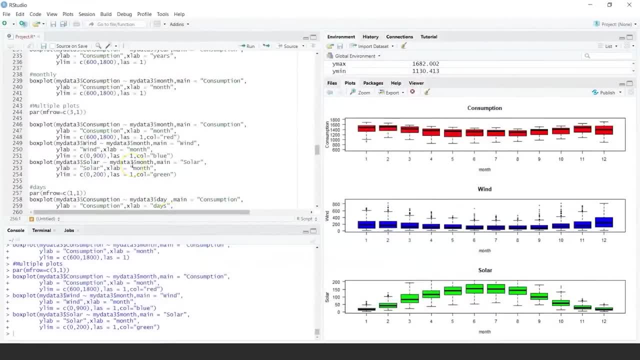 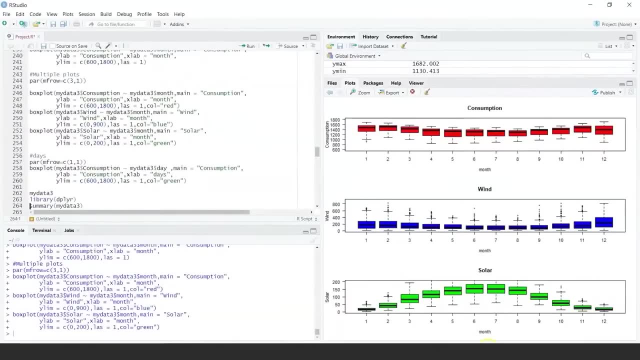 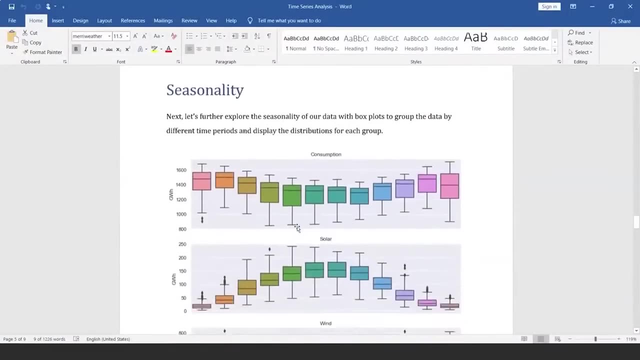 box plots which are giving us values. now, what I can also do is I could look at the day wise also, but before we look into this, how do I infer some information from these box plots which are being created? so this is what we have done, where we are looking at. 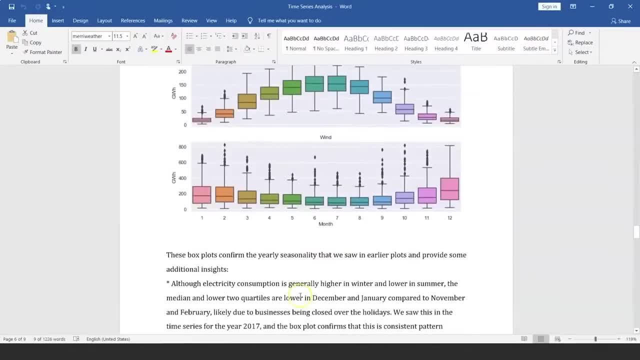 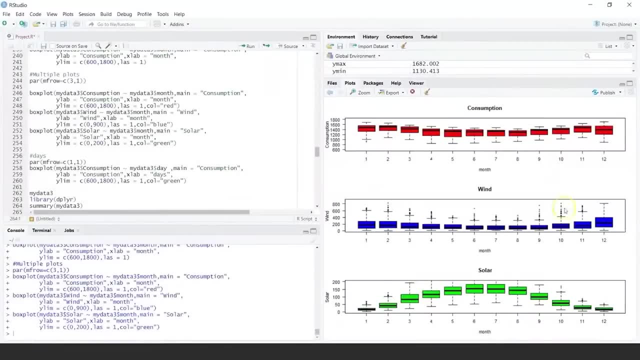 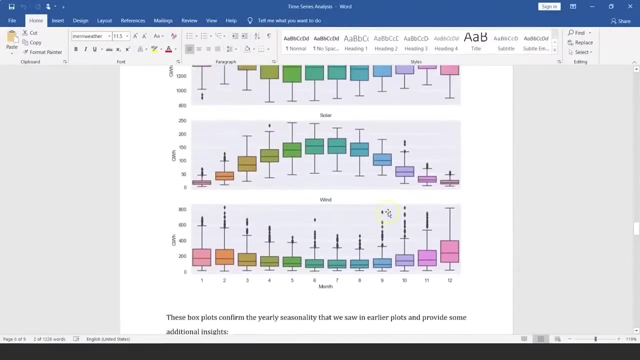 the data for month. and these box plots give me year seasonality, which we were seeing in earlier plots, but give some additional insights. so if I look at the data here, it tells me the electricity consumption is generally higher in winter. now this is based on months, so we can see consumption. 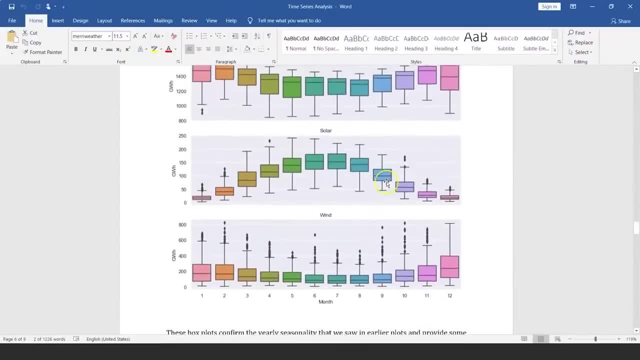 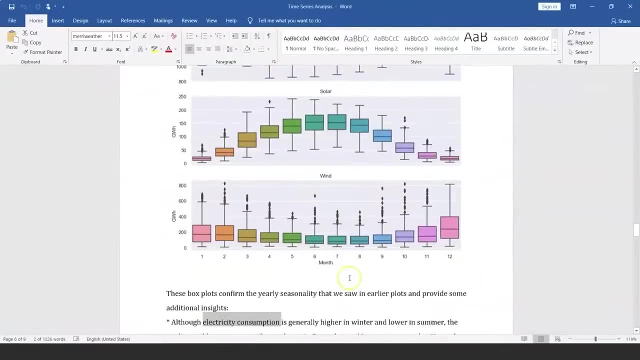 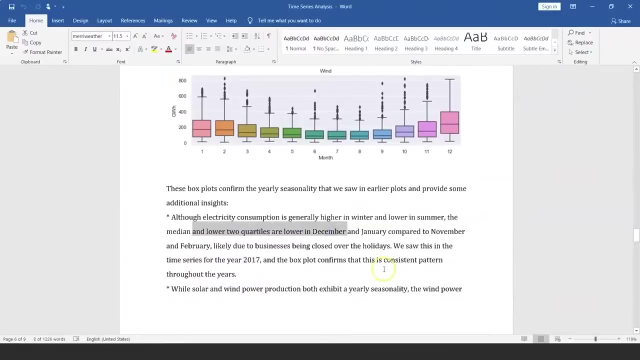 is higher in winters and lower in summer. so we can obviously look at our plot. we can see where it is lower, where it is higher, and then we can look at the median and lower. two quartiles are lower in December and January compared to November and February. 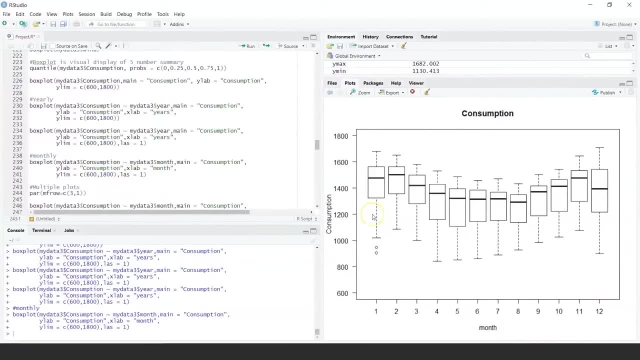 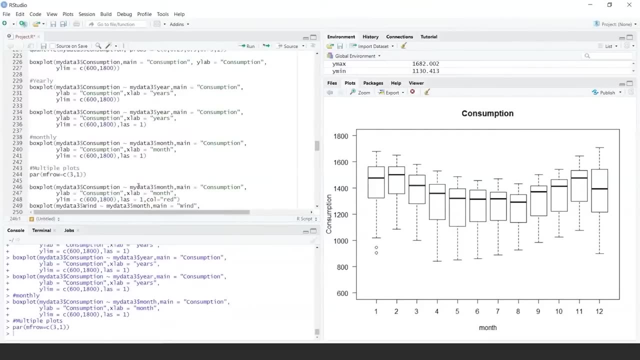 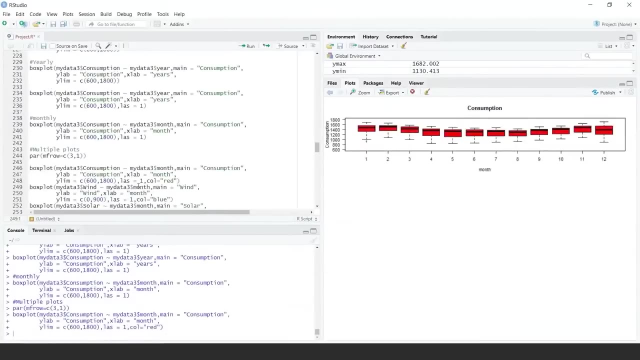 particular year, or i can just do a grouping based on months so i can have multiple plots to see a difference here. so lets do this now. lets create a box plot for consumption, which is monthly data, and lets give it a color. lets look at the wind data, which is again grouped monthly. 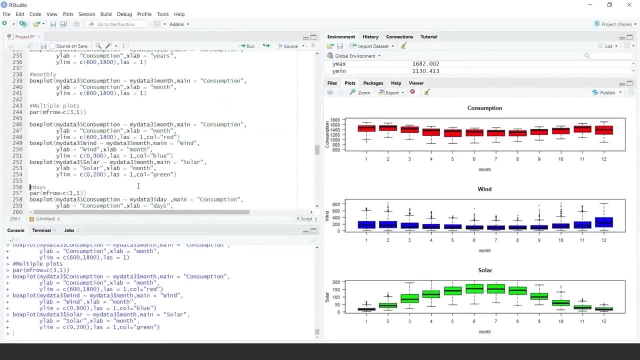 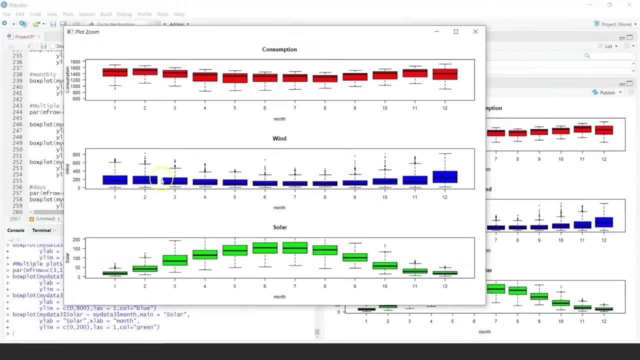 and lets look at the solar data, which is grouped monthly. now, if i zoom in, it basically gives me the seasonality of the data for your wind, for your consumption, for your solar. so what we are doing is we are creating these box plots which are giving us values. 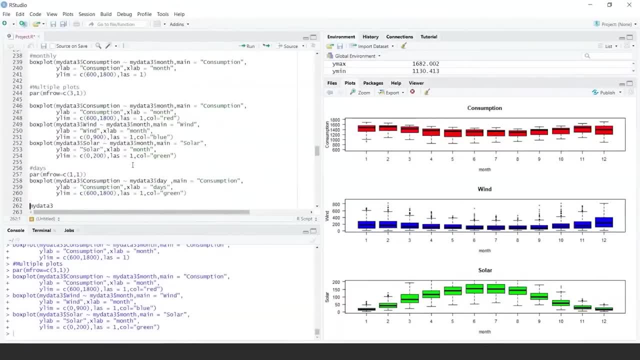 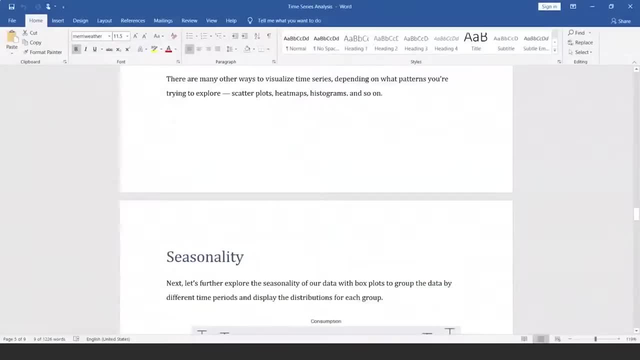 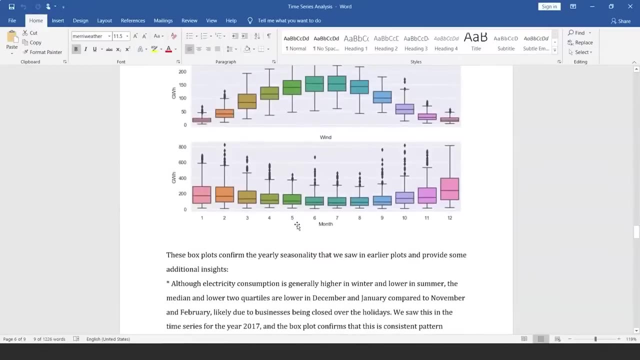 now, what i can also do is i could look at the day wise also, but before we look into this, how do i infer some information from these box plots which are being created? so this is what we have done, where we are looking at the data for month and 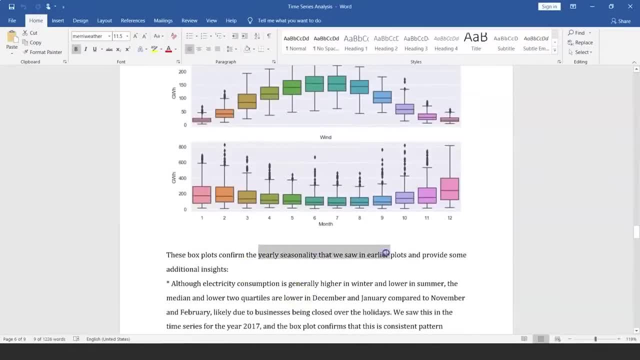 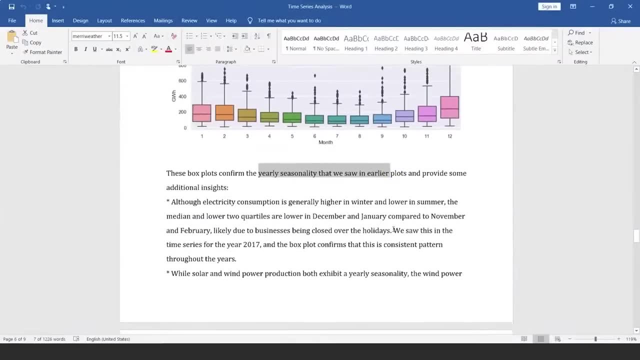 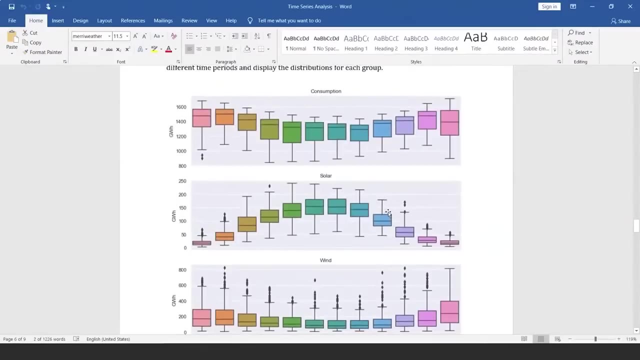 these box plots give me year seasonality, which we were seeing in earlier plots, but give some additional insights. so if i look at the data here, it tells me the electricity consumption is generally higher in winter. now this is based on months, so we can see consumption is higher. 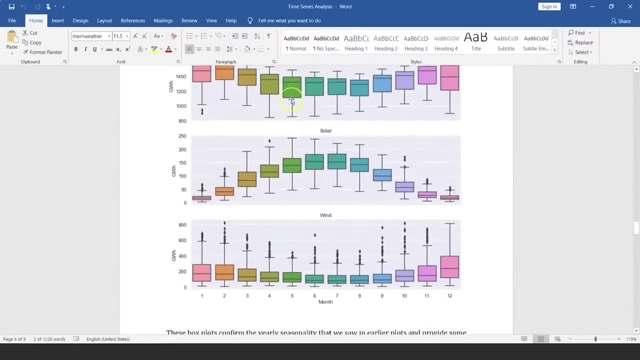 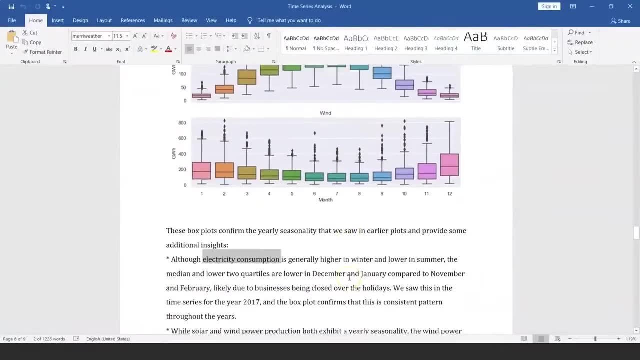 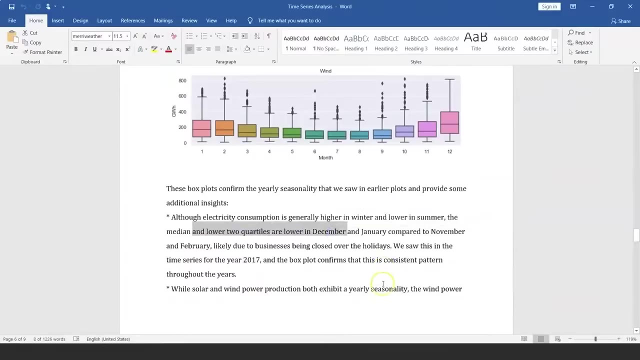 in winters and lower in summer. so we can obviously look at our plot. we can see where it is lower, where it is higher, and then we can look at the median and lower. two quartiles are lower in december and january compared to november and february. 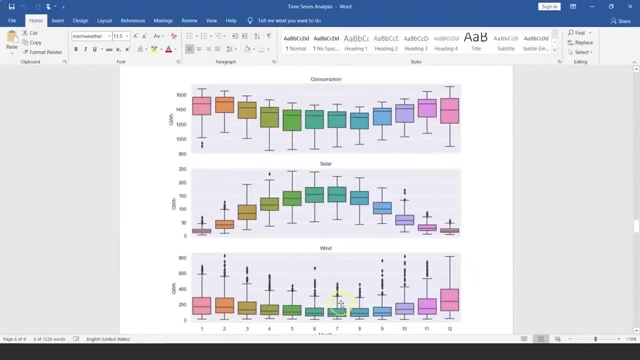 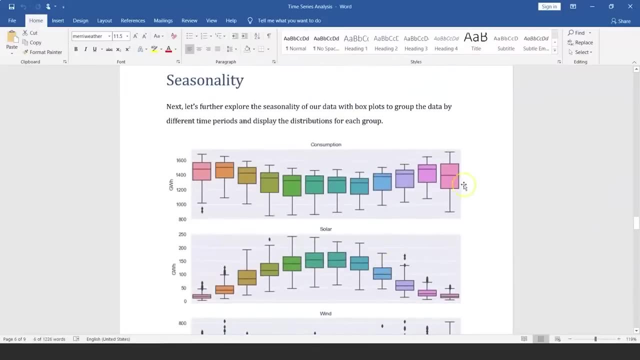 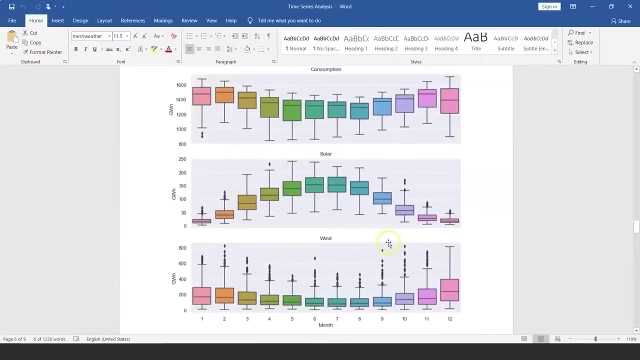 so that is, you look at the quartiles and you will see that the median and lower two quartiles are lower in december and january. here jan and december. so you can look at from my plot. now this is giving you some idea on seasonality. now 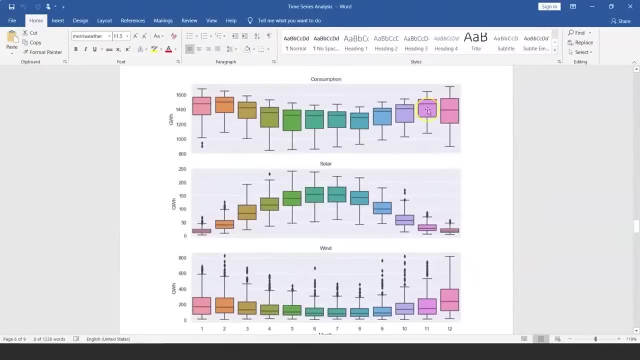 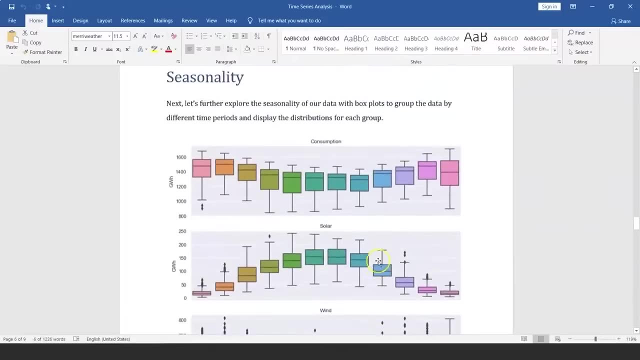 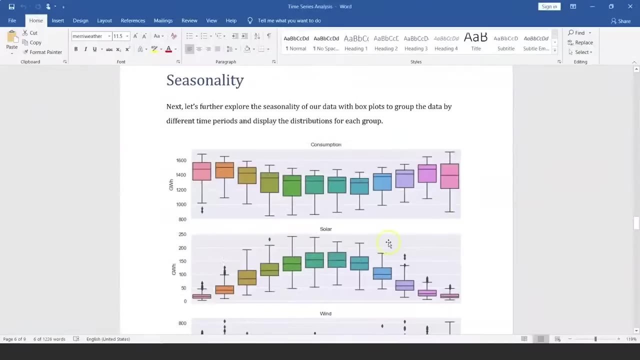 so that is, you look at the quartiles and you will see that the median and lower two quartiles are lower in December and January. here Jan and December. so you can look at from my plot. now this is giving you some idea on seasonality. now that might be due. 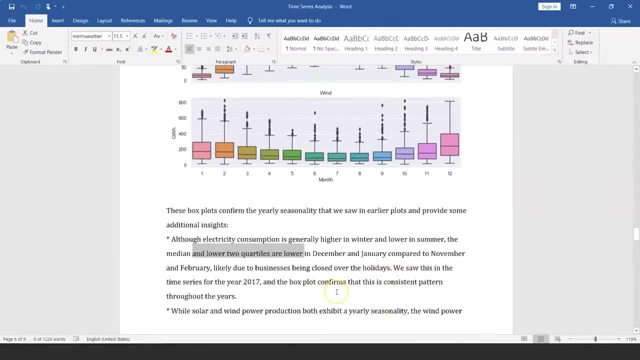 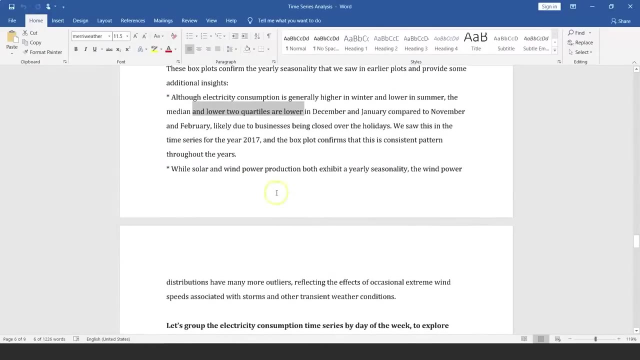 to business being closed over holidays. now this one we were also seeing when we looked at time series for 2017 only, and box plot basically confirms that there is this consistent pattern throughout the years. now, when you look at your solar and wind power production, both will 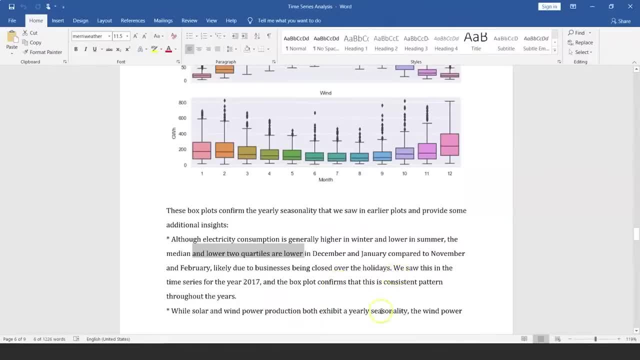 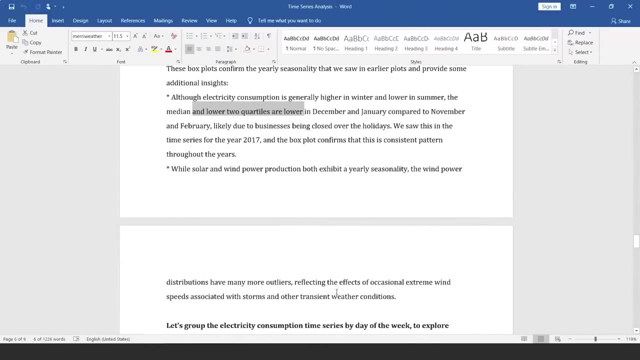 that might be due to business being closed over holidays. now, this one we were also seeing when we looked at time series for 2017 only, and box plot basically confirms that there is this consistent pattern throughout the years. now, when you look at your solar and wind power, 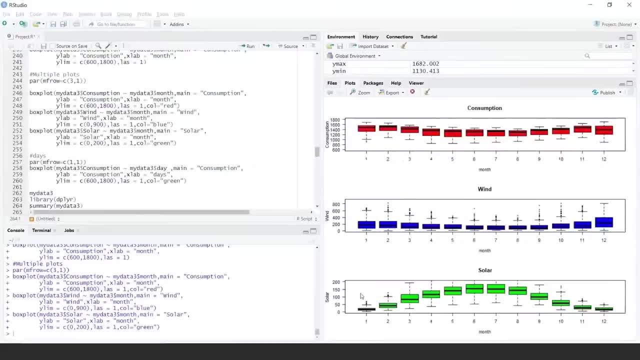 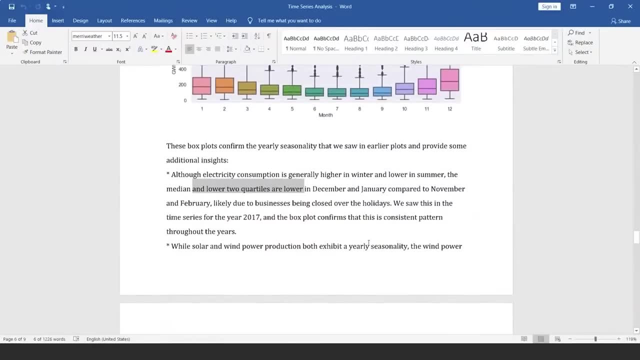 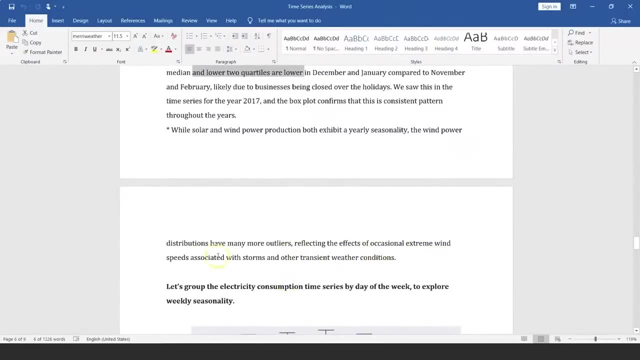 production. both will give you a year seasonality, what we are seeing here and if, basically, i look at the data, so it depends on what parameters you are choosing. but if you look at solar, it will reflect the effect of occasional extreme wind speeds associated with storms and other transient. and since we 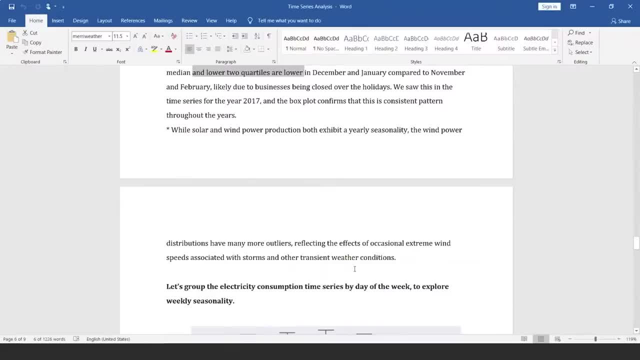 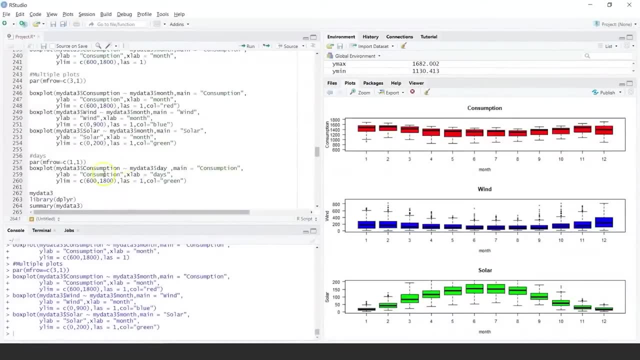 are grouping it based on months, we can see this pattern is quite evident every year. now what we can do is we can group the data day wise. so here let me again reset this to one plot per graph. now i will say box plot, i will say consumption, which is 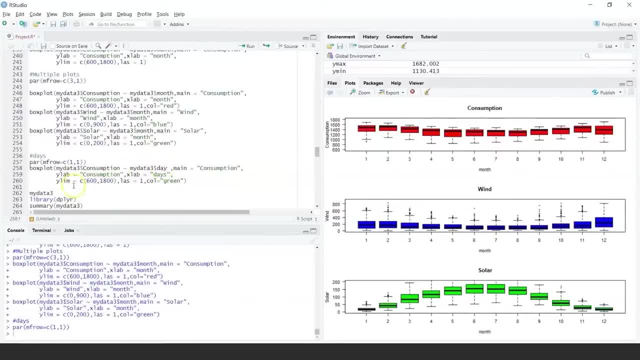 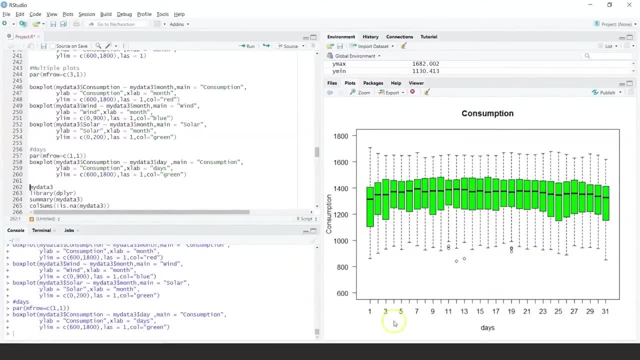 group based on day. now we know that there is a day column and lets give a while limit and lets look at the data. so this is where i am grouping the data day wise. so you look at 31 days and you look at the box plot. so this is where you are. 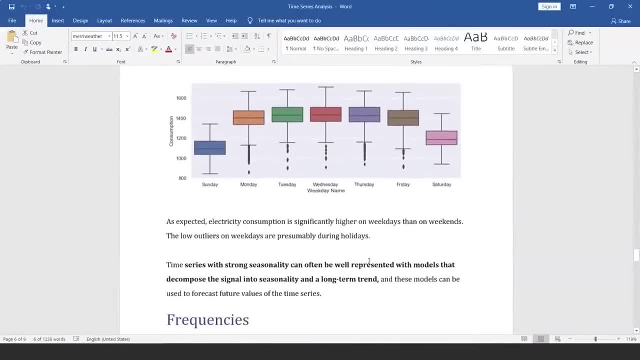 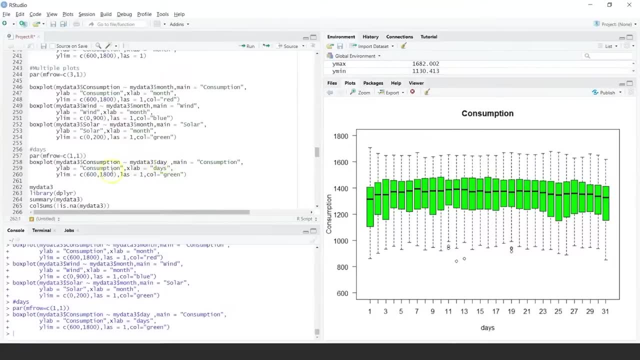 plotting it on a daily basis so you can look at the data. you can break it down to a particular week. so here i have given day and i have chosen all the 31 days, but i can break it down to a week and i can look at the data. so 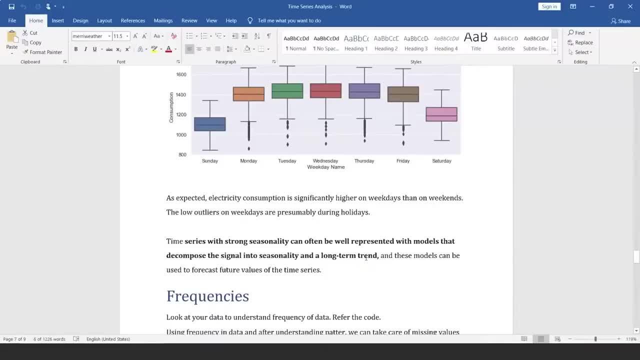 if we look at the data per week or per day, we can basically infer that electricity consumption, where i am doing a consumption group by day, is higher on week days than on weekends. so time series with strong seasonality can often be represented with models that can decompose signal into 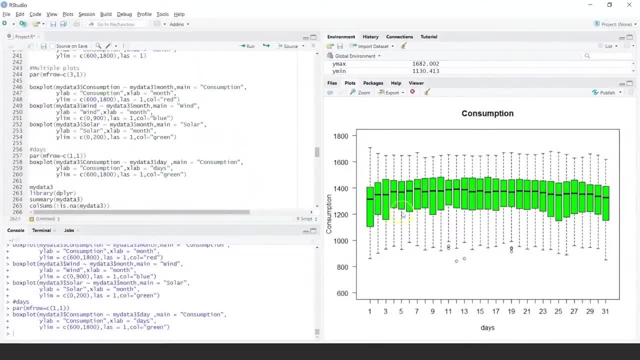 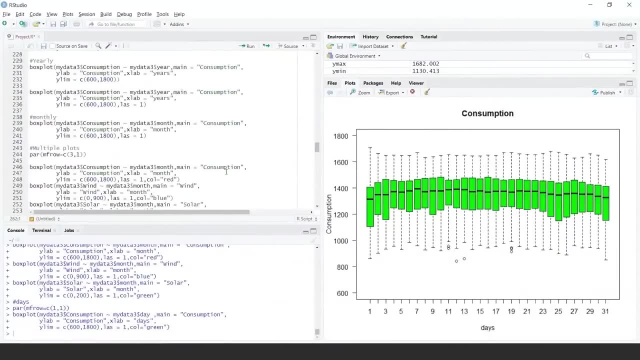 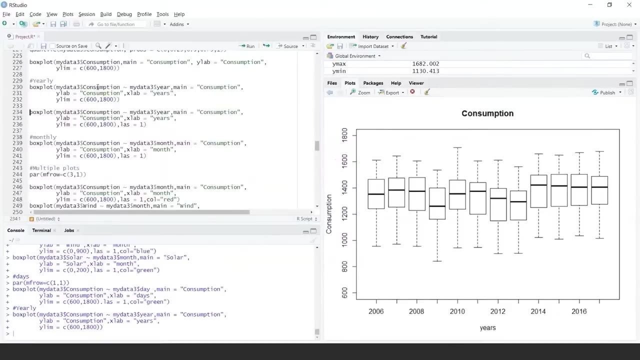 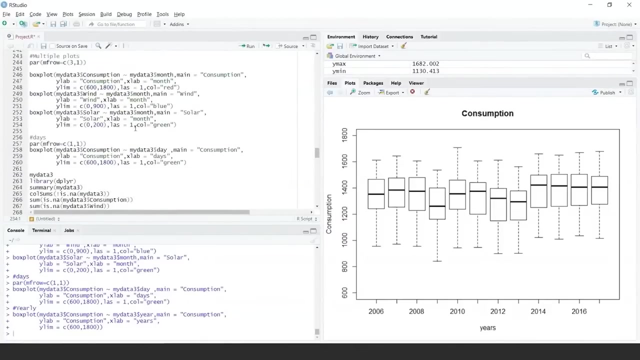 seasonality and long trend. now, this is an easy way. now, how do we look at the frequency of the data that could be interesting to see? so let me look at, say, the yearly data which we were seeing here. now lets go further, and here we have looked at data. so what we will do? 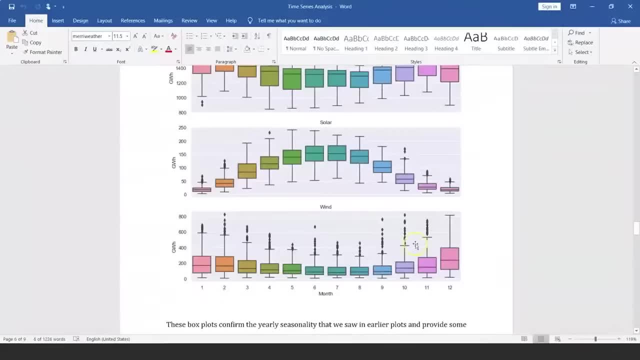 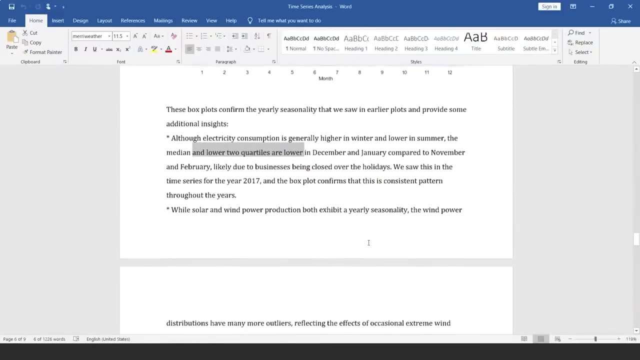 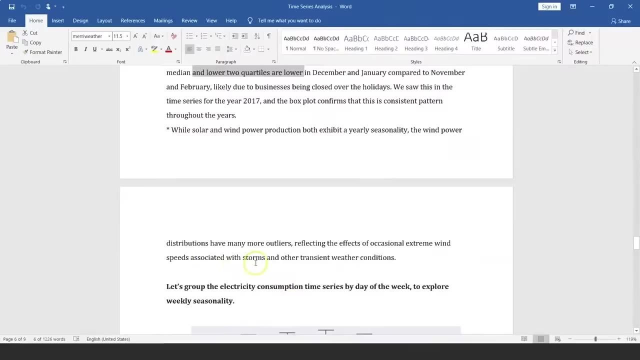 give you a year seasonality, what we are seeing here and if, basically, I look at the data, so it depends on what parameters you are choosing. but if you look at solar, it will reflect the effect of occasional extreme wind speeds associated with storms and other transient and. 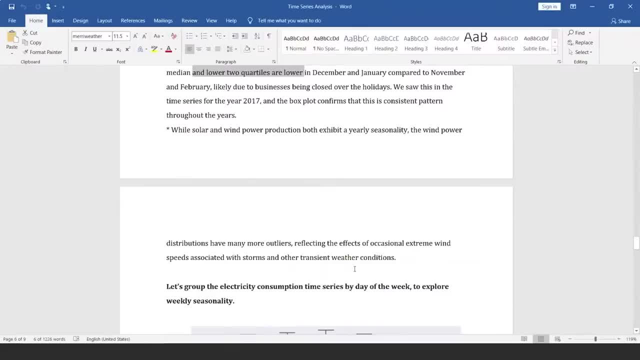 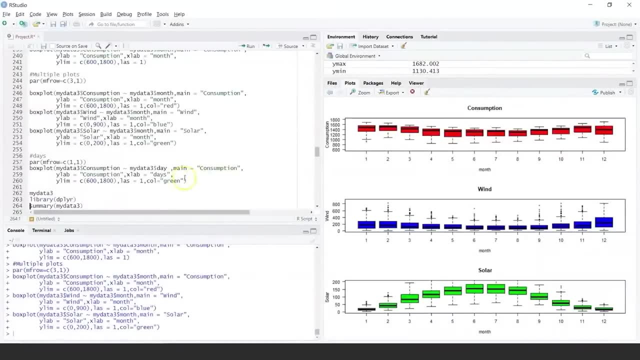 since we are grouping it based on months, we can see this pattern is quite evident every year. now what we can do is we can group the data day wise. so here let me again reset this to one plot per graph. now I will say box plot, I will say consumption. 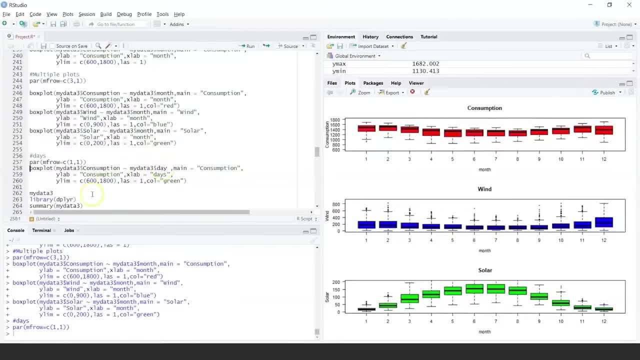 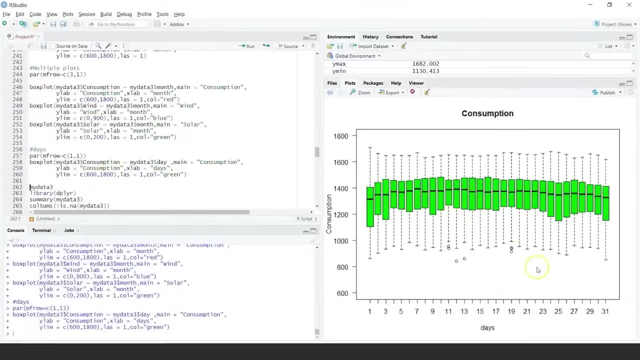 which is group based on day. now we know that there is a day column and let's give a while limit and let's look at the data. so this is where I am grouping the data day wise. so you look at 31 days and you look at the box. 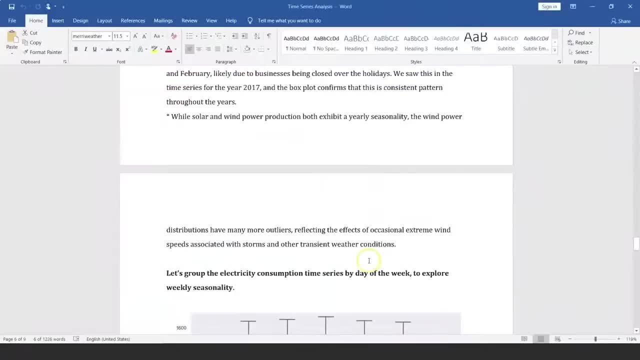 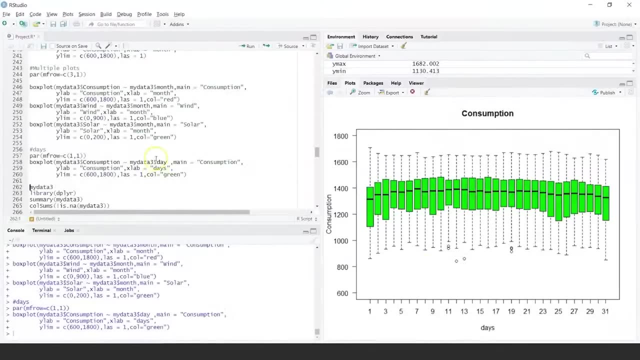 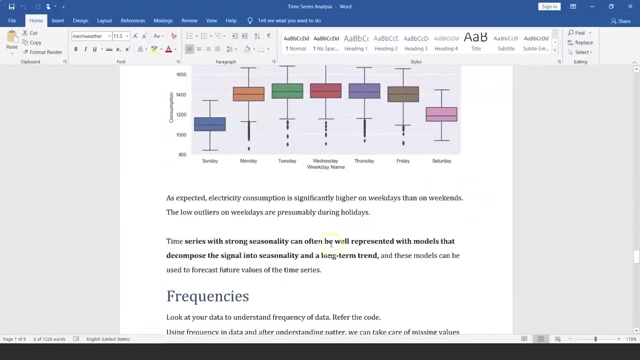 plot. so this is where you are plotting it on a daily basis, so you can look at the data. you can break it down to a particular week. so here I have given day and I have chosen all the 31 days, but I can break it down to a week and I can look at the. 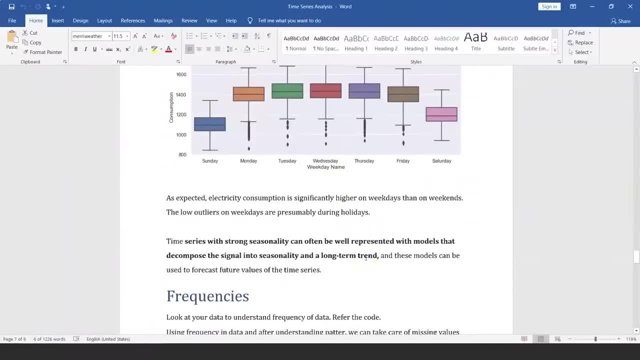 data. so if we look at the data per week or per day, we can basically infer that electricity consumption, where I am doing a consumption group by day, is higher on week days than on weekends. so time series with strong seasonality can often be represented with models that. 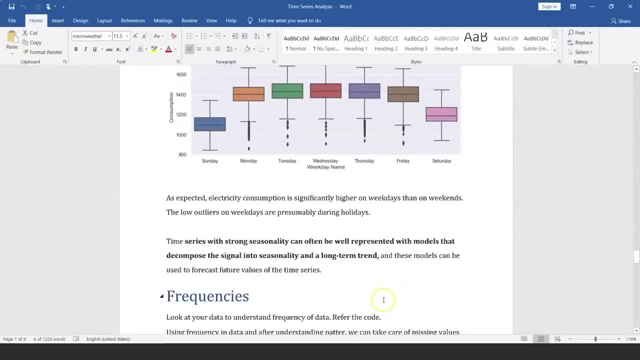 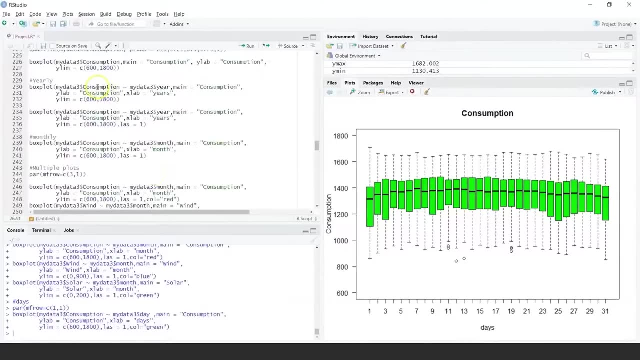 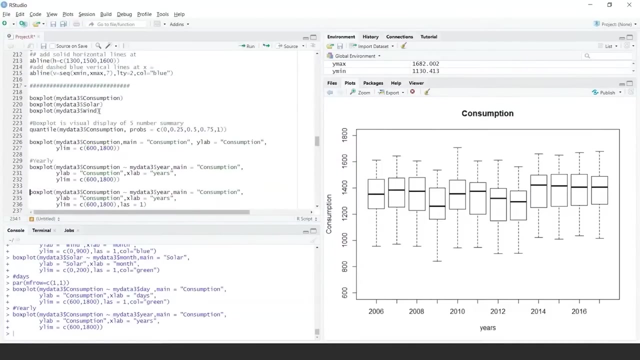 can decompose signal into seasonality and long trend. now, this is an easy way. now, how do we look at the frequency of the data that could be interesting to see? so let me look at, say, the yearly data which we were seeing here. now let's go further, and here: 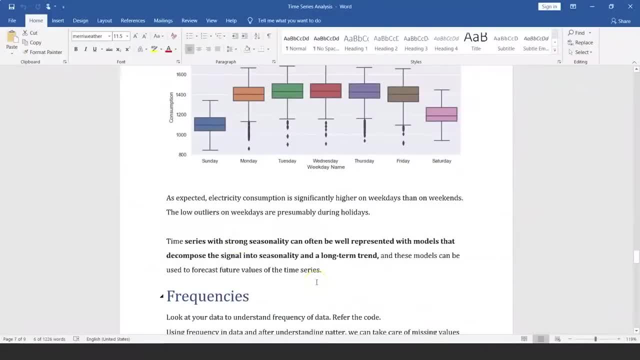 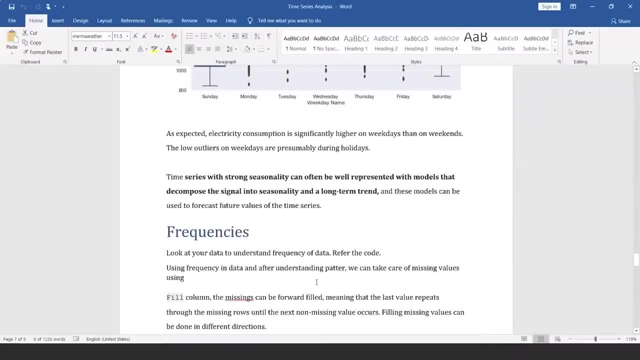 we have looked at data. so what we will do is we look at the frequency. now, when you look at the frequency, when you talk about frequency in your data, so we have the modified date column which gives me a frequency, and if we really look into the data, that will tell me. 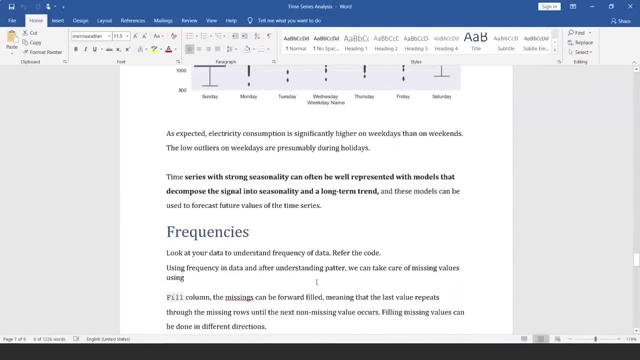 is: we look at the frequency. now, when you look at the frequency, when you talk about frequency in your data, so we have the modified date column which gives me a frequency and if we really look into the data, that will tell me that the data is on a 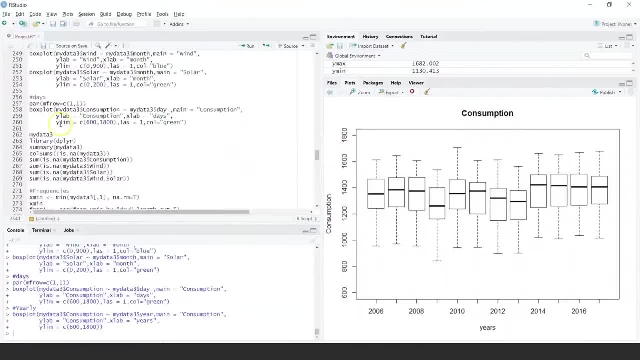 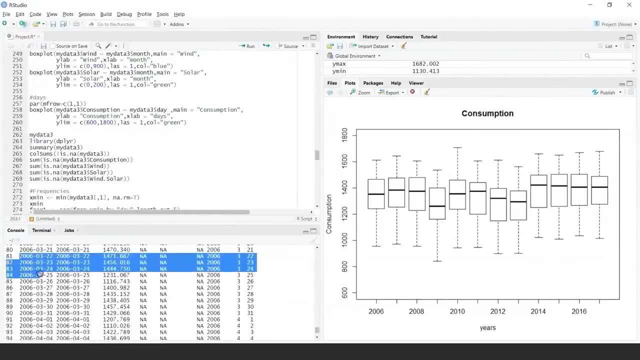 that the data is on a daily basis. so for that let's look at my data 3 again, which gives me data, and you can just see all the data or dates are in sequence, so your 22, 23, 24, 25, 26 and so. 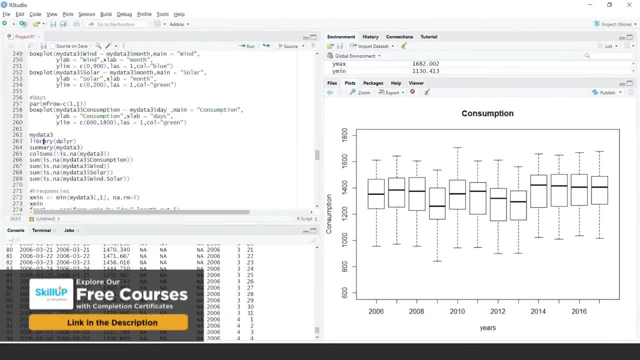 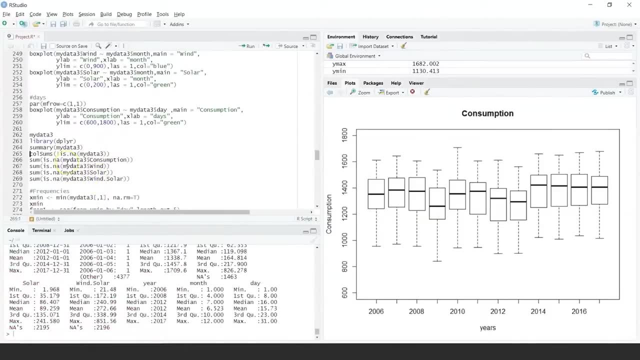 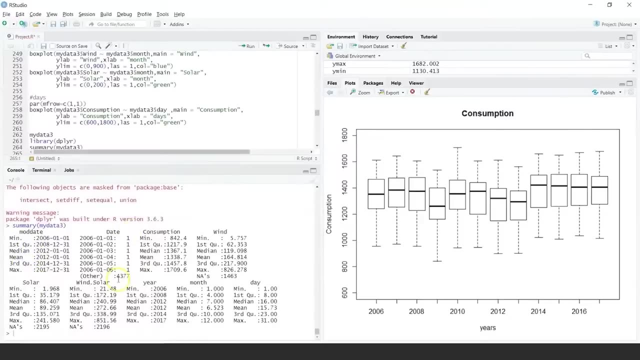 on. I can look at. I can access a dplyr package that is basically allowing me to work in a better way. now I can look at the summary of this and for all my columns I am seeing what is the minimum 5 number, summary date and consumption. so date does not show me anything. 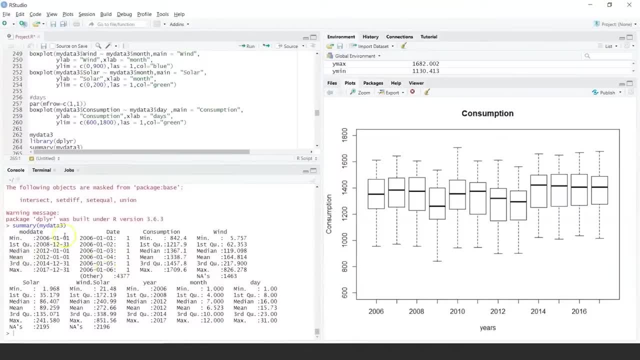 because this is not in a date format, it is just a factor. but other things have the 5 number summary. so we are looking at win plus solar, we are looking at year and month and day and all these columns. now what we will do is we will. 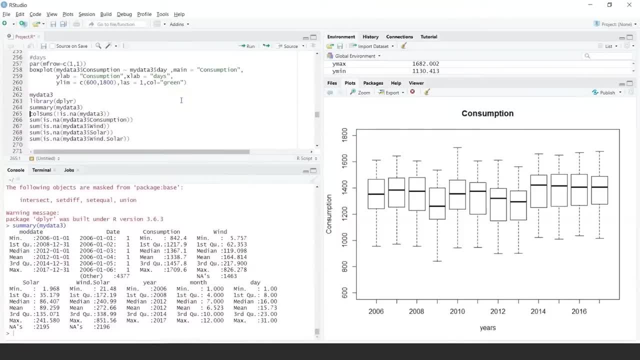 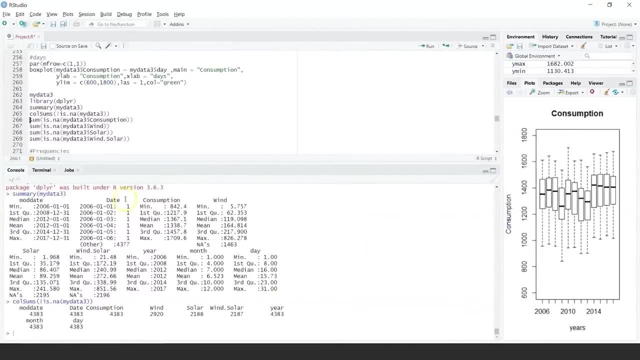 want to find out the sum of each column, how many entries does it have, and we will say the value, should any value should not be considered. so let's look at this one, so it tells me for my particular columns. so let me run this again and that 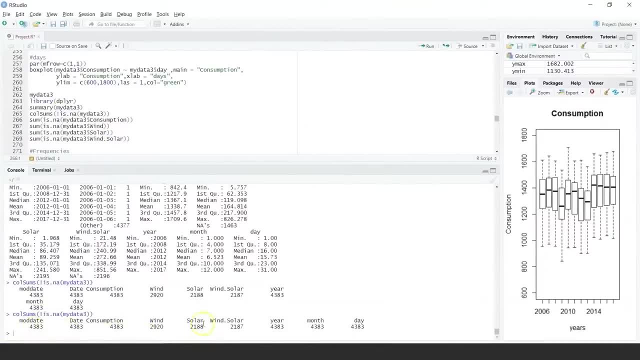 shows me for each column how many values you have, and these counts do not include the NA values. now, similarly, I can find out specifically for consumption. I can find out: is there any NA value? so I am saying: is dot NA and let's find out if there. 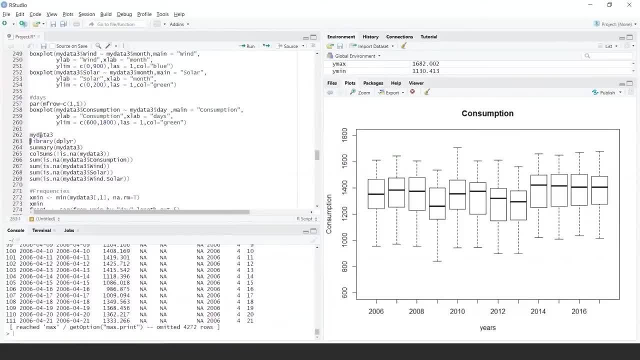 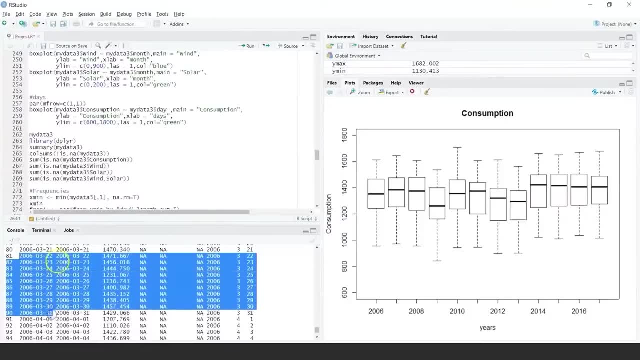 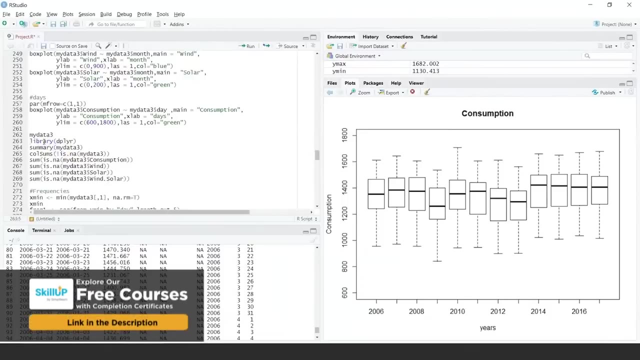 daily basis. so for that, lets look at my data 3 again, which gives me data and you can just see all the data or dates are in sequence. so your 22, 23, 24, 25, 26 and so on i can look at. i can access a dplyr package. 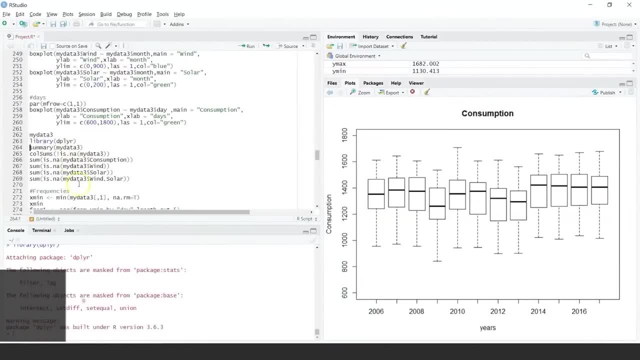 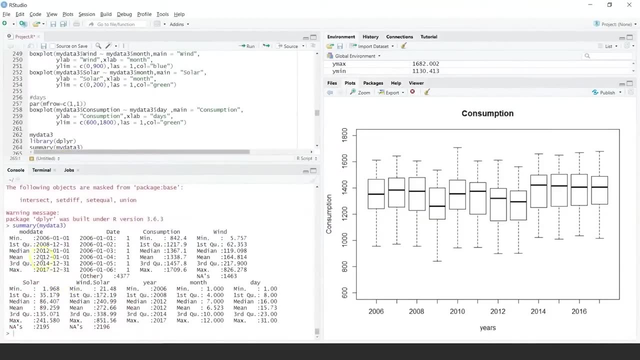 that is basically allowing me to work in a better way. now i can look at the summary of this and for all my columns i am seeing what is the minimum 5 number, summary date and consumption. so date does not show me anything because this is not in a date format. it is. 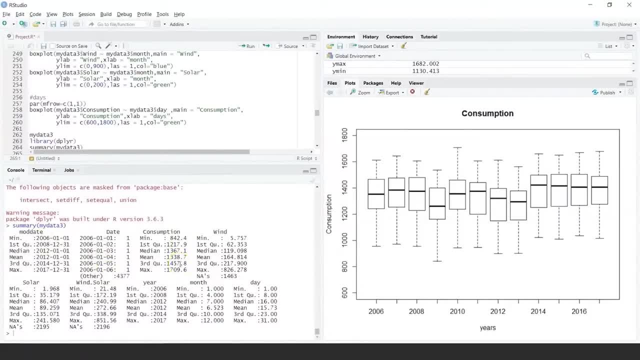 just a factor, but other things have the 5 number summary. so we are looking at wind plus solar, we are looking at year and month and day and all these columns. now what we will do is we will want to find out the sum of each column, how many. 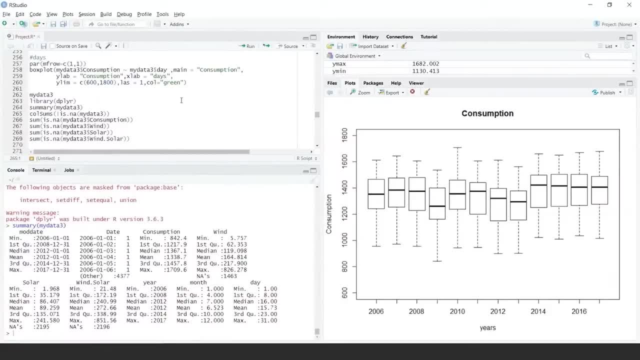 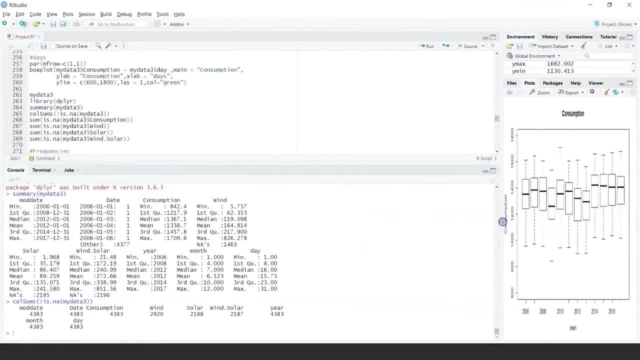 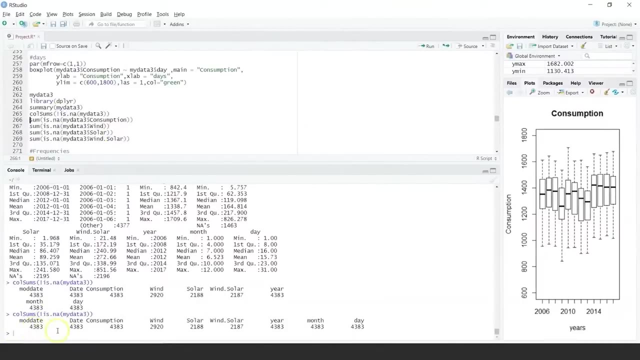 entries does it have? and we will say: the value should NA value should not be considered. so lets look at this one. so it tells me for my particular columns, so let me run this again and that shows me for each column how many values you have and these counts. 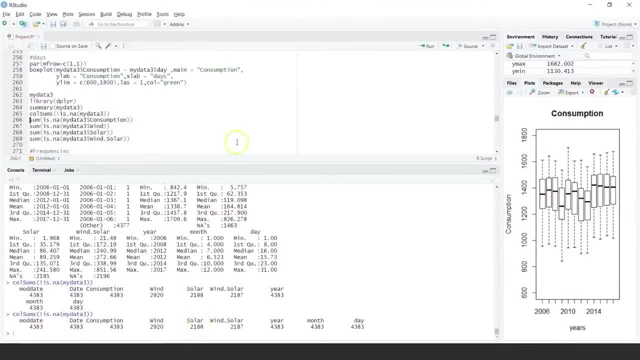 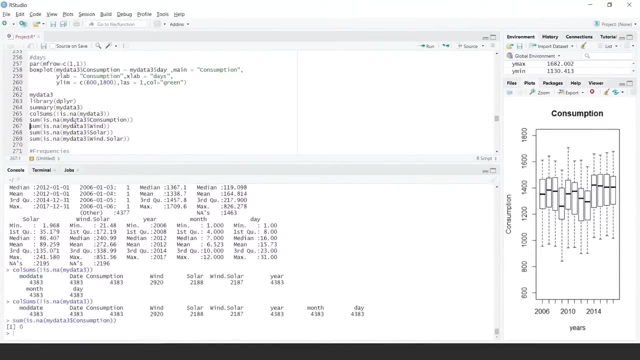 do not include the NA values now. similarly, i can find out specifically for consumption. i can find out: is there any NA value? so i am saying: is dot NA and lets find out if there is any NA value or missing value in consumption. it says 0. ok, thats good. 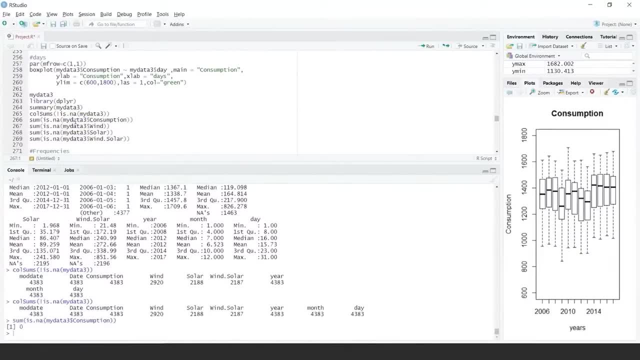 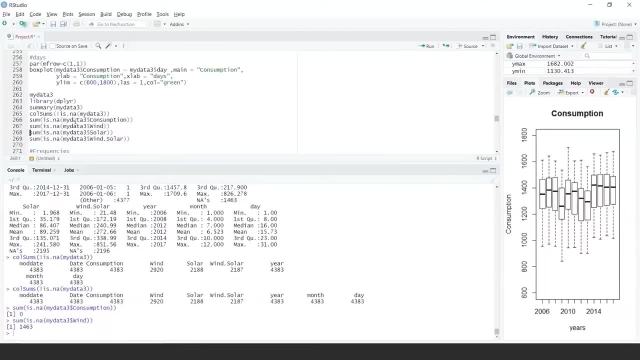 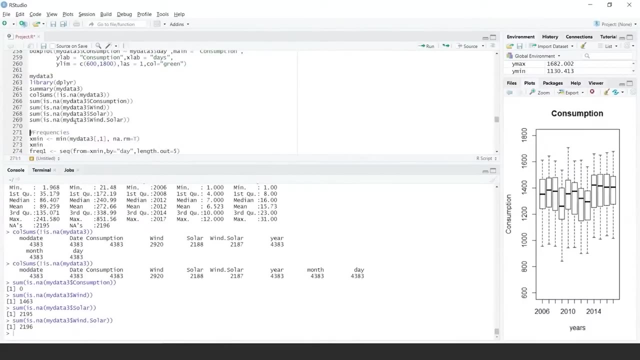 is any NA value or missing value in consumption? it says 0. ok, that's good. if you look in wind, it tells me there are 463 entries which are NA, similarly solar, similarly wind, dot solar or wind plus solar. so it gives me a count of NA. 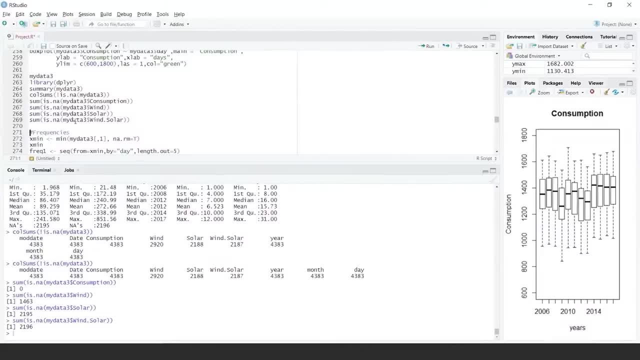 values, that is, missing values and also values which are not missing. so, to understand frequency, what we can do is we can find out the minimum on the date. that is the first column, and I am saying RM, NA dot. RM is true, that is, get rid of NA values. 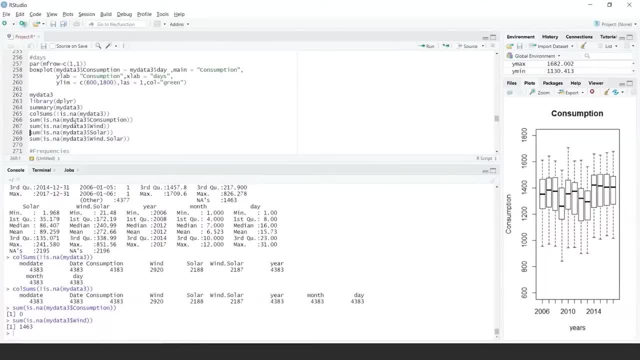 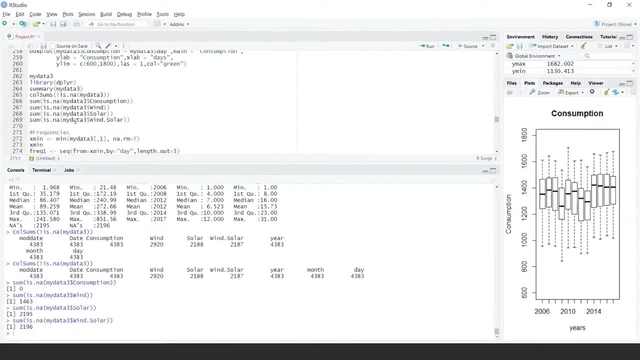 if you look in wind, it tells me there are 1463 entries which are NA, similarly solar, similarly wind, dot solar or wind plus solar. so it gives me a count of NA values, that is, missing values and also values which are not missing. so to understand frequency, 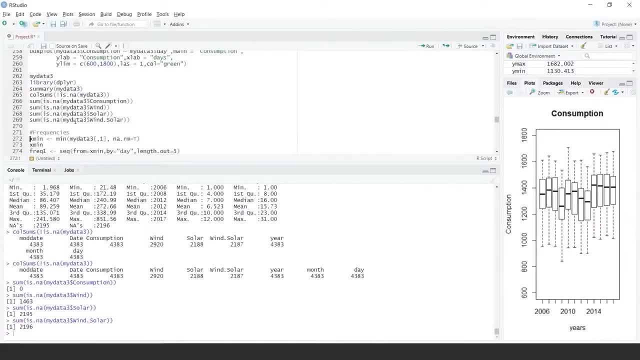 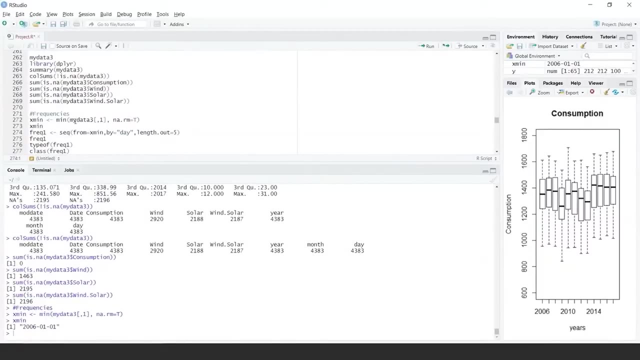 what we can do is we can find out the minimum on the date. that is the first column, and i am saying rm, NA dot. rm is true. that is, get rid of NA values and find out the minimum and lets look at the minimum value. this is the minimum from my modified date. 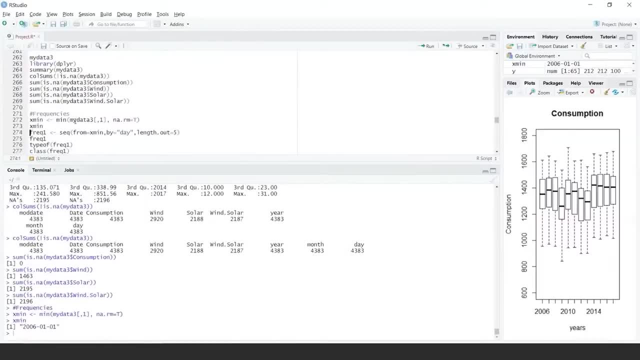 and find out the minimum. and let's look at the minimum value. this is the minimum from my modified date. now if I would want to get the frequency, I can basically use sequence function so I can say: from X, minimum, that is the minimum value. I want to look at the frequency. that is day. 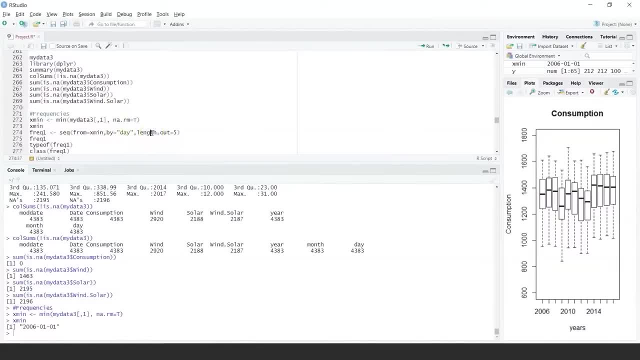 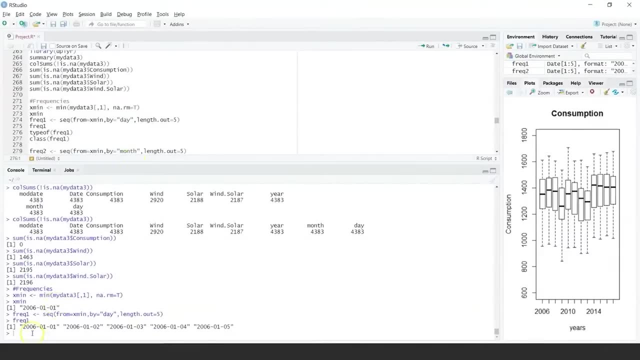 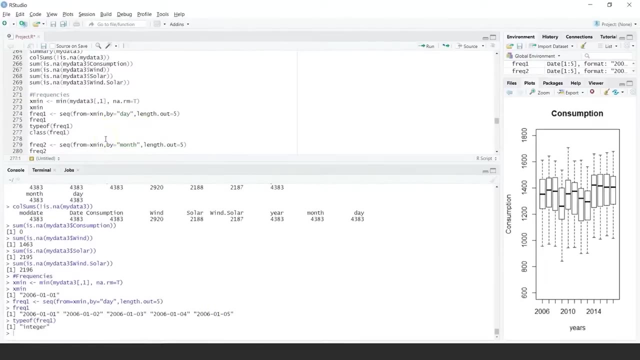 wise and let's just look at 5 entries and see if there is a day by day frequency. so let's look at the value of this and obviously it tells me there is day wise frequency. so that allows me to look at the frequency, look at the type of it. 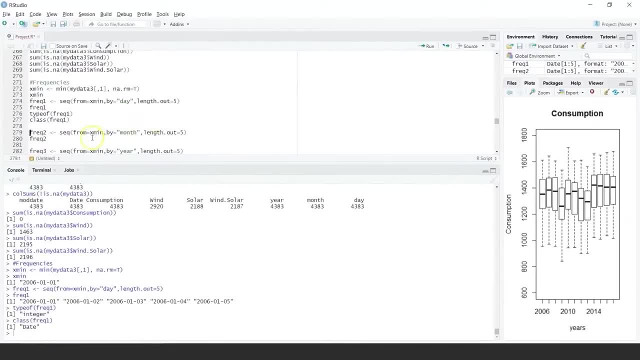 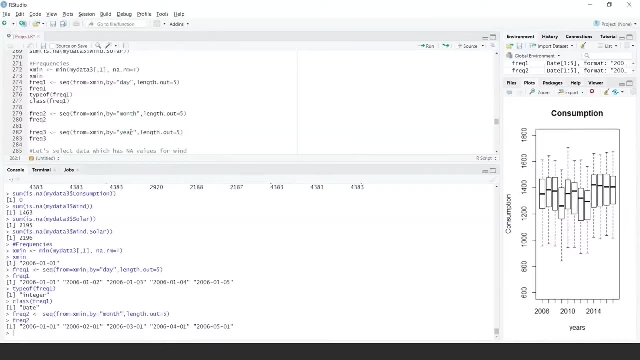 it is an integer class, is a date. so similarly we can say: from X minimum we can basically look at the frequency month wise, and I can again look at 5 records. so that shows me monthly data right, so I can extract the data for frequency, similarly yearly data, and that's also. 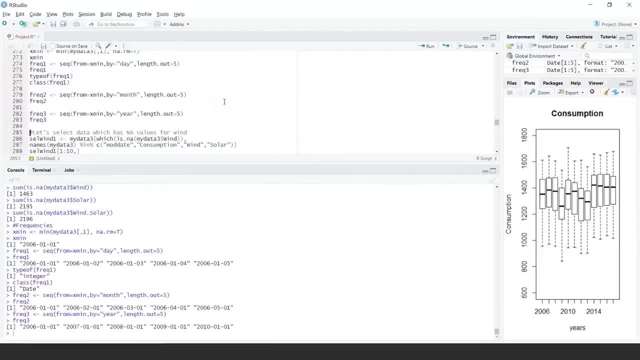 very useful. now we can select data which has NA values for wind. so how do I do it? I would want to find out the wind column and I want to find out where the values are NA. so I will create a variable and here I will say my data. 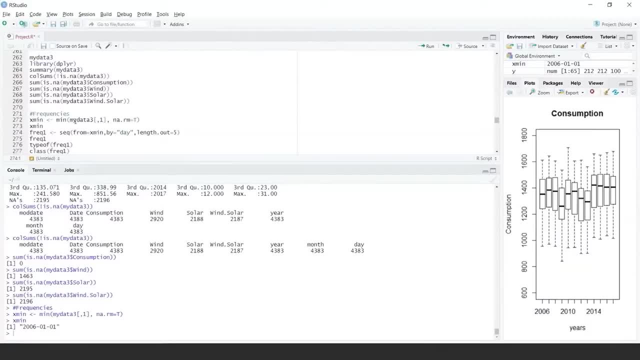 now, if i would want to get the frequency, i can basically use sequence function so i can say: from x, minimum, that is the minimum value. i want to look at the frequency. that is day wise, and lets just look at 5 entries and see if there is a day by. 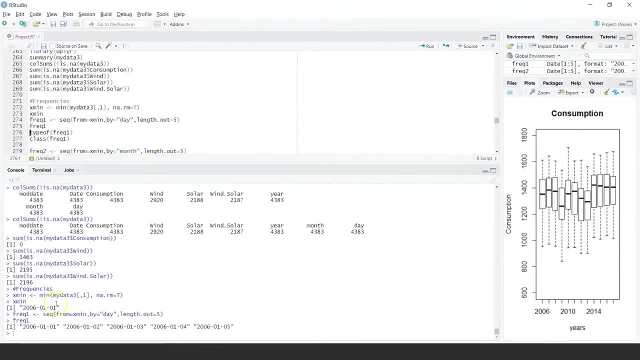 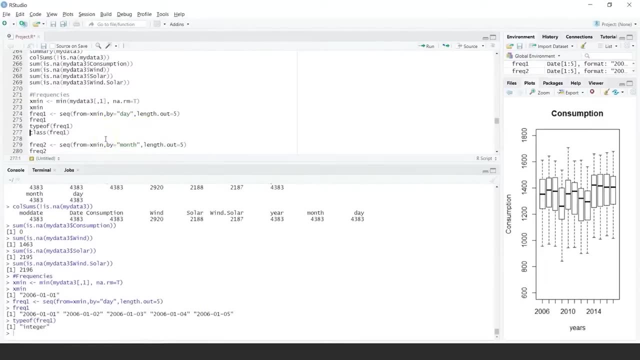 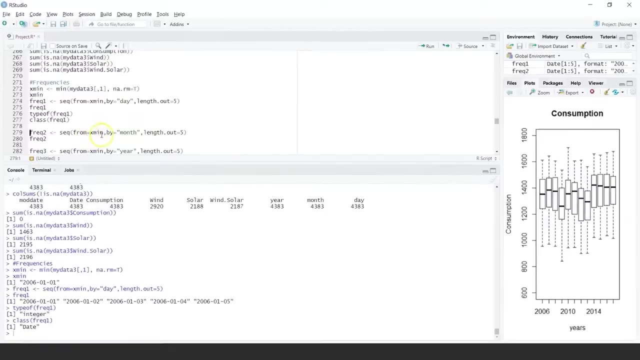 day frequency. so lets look at the value of this. and obviously it tells me there is day wise frequency. so that allows me to look at the frequency. look at the type of it. it is an integer class, is a date. so similarly we can say: from x minimum, we can basically look at. 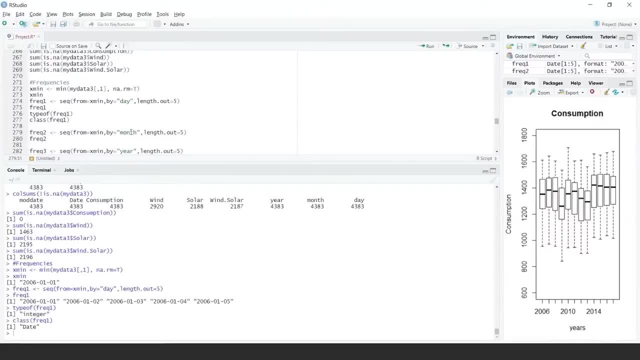 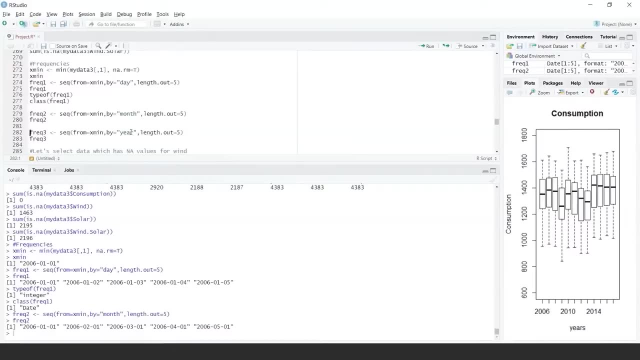 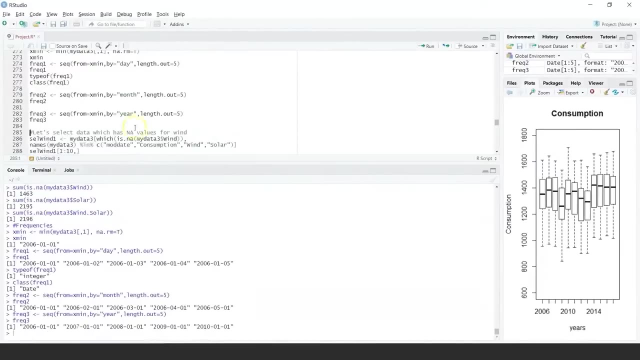 the frequency month wise, and i can again look at 5 records. so that shows me monthly data right, so i can extract the data for frequency, similarly yearly data, and thats also very useful. now we can select data which has NA values for wind. so how do i do it? i would want to. 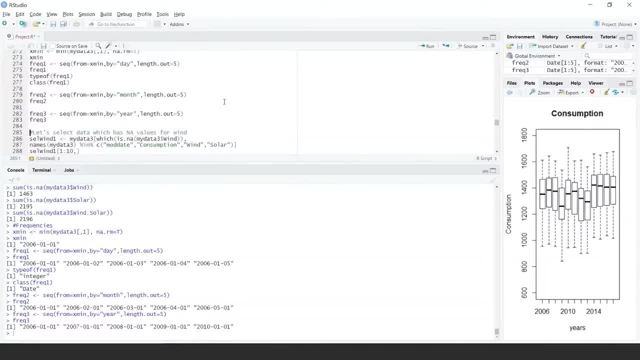 find out the wind column and i want to find out where the values are NA. so i will create a variable and here i will say my data 3 and then i give a conditional where i say is NA in the column. so lets do this now. once i have done this, 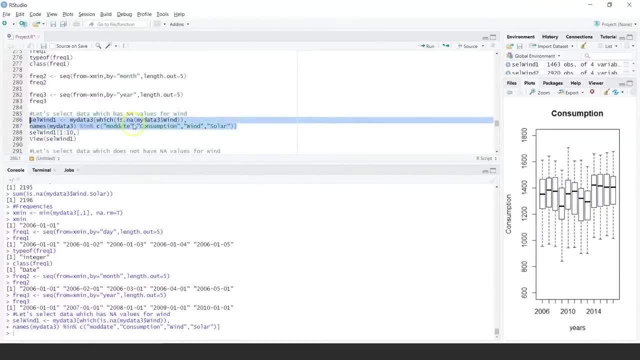 once i have done this. i have said that my selected wind data from my data 3 where we said NA values, and i will give the names to this. so name should be in my data 3. i am interested in mod data consumption- wind and solar. so these are the 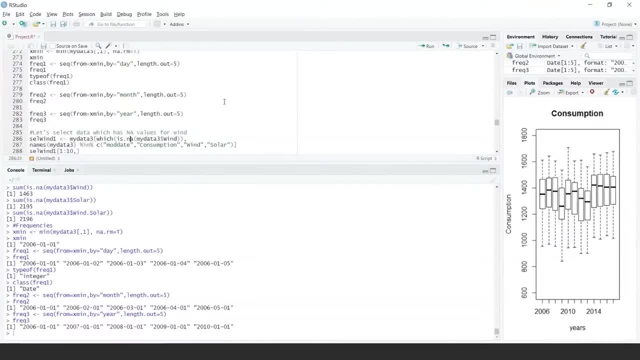 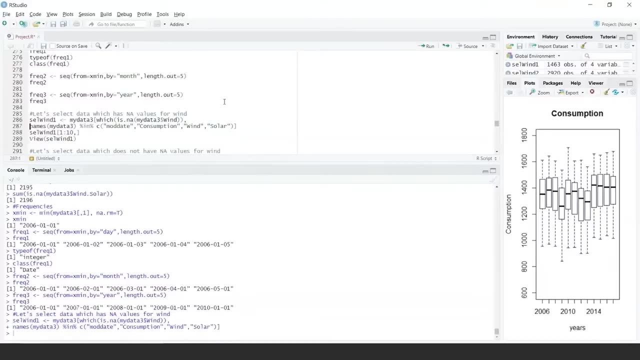 3 and then I give a conditional where I say: is NA in the column? so let's do this now. once I have done this, once I have done this, I have said that my selected wind data from my data 3, where we said NA values and 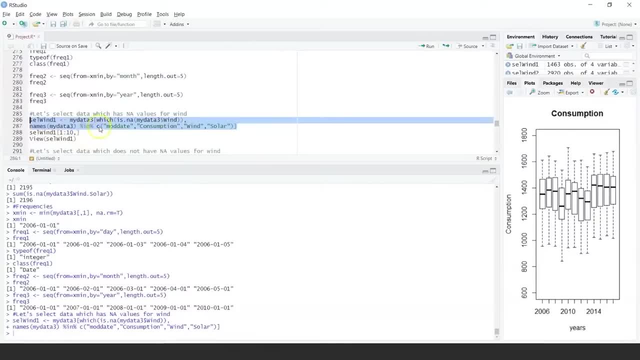 I will give the names to this, so name should be in my data. 3: I am interested in mod data consumption, wind and solar. so these are the 4 columns I am interested in. let's look at first 10 records here, or first 10 rows. so 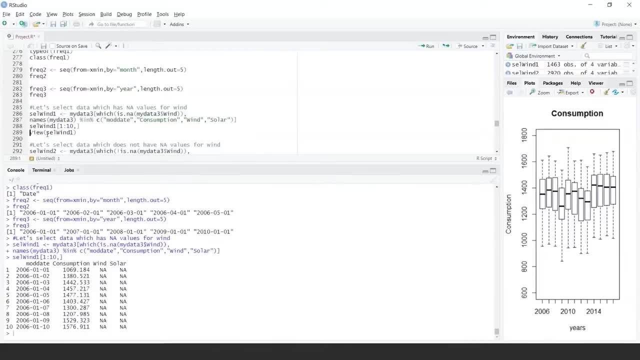 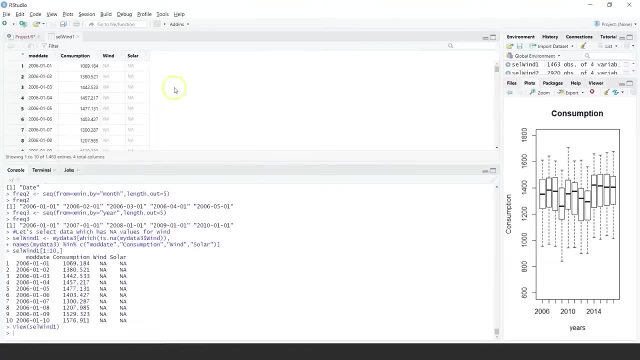 that tells me these are the values. where wind has NA or missing values, I can always do a view and that gives me the complete data. so it basically shows me 1463 entries and here it shows me all NA values. so you can look at all the way to the end. 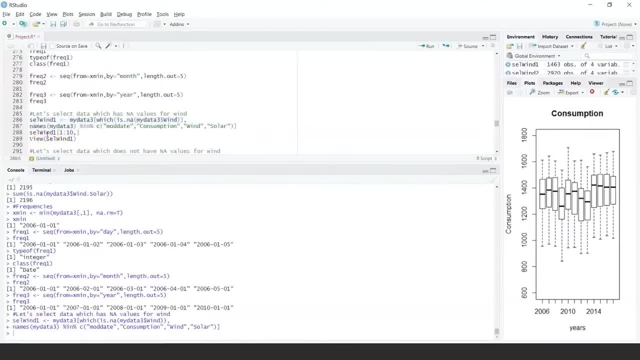 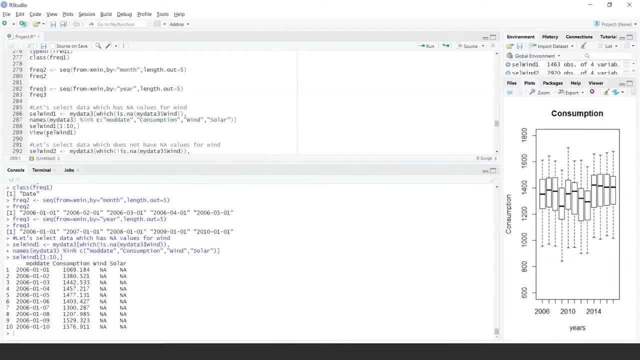 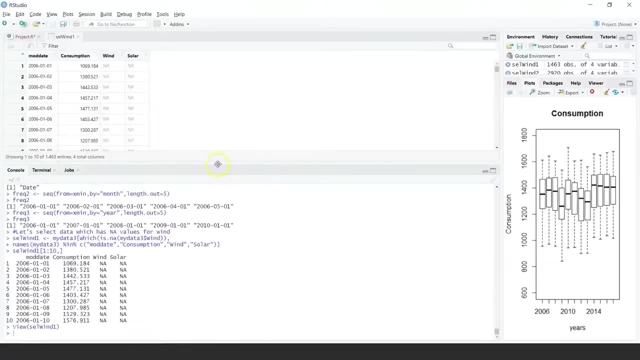 4 columns i am interested in. lets look at first 10 records here, or first 10 rows. so that tells me these are the values. where wind has NA or missing values, i can always do a view and that gives me the complete data. so it basically shows me. 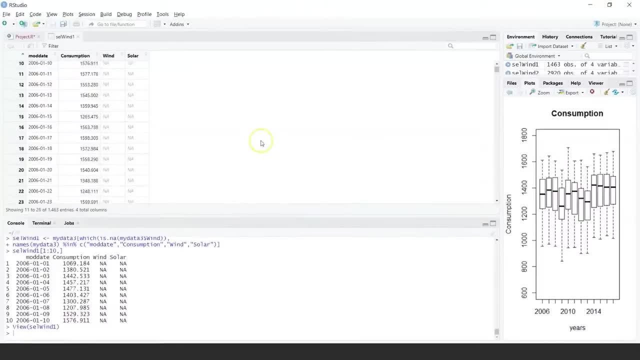 1463 entries and here it shows me all NA values, so you can look at all the way to the end, and it shows me wind has NA, solar does have some value, here in the last row, but then also, if you see, the numbers have a difference. so 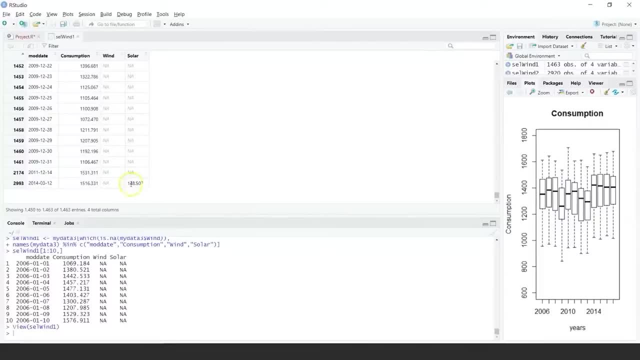 and it shows me wind has. NA solar does have some value here in the last row, but then also, if you see the numbers, you will have a difference. so you have 1461 and then you have 2174. so there is a difference. so there is some. 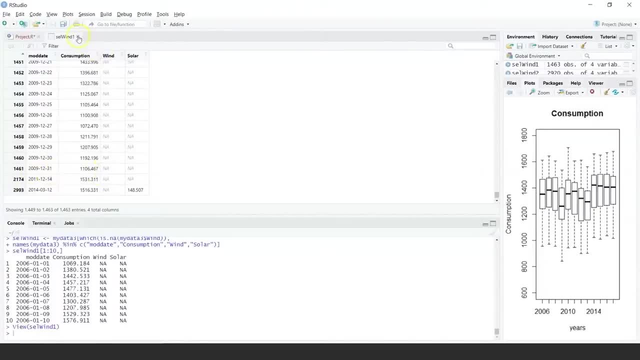 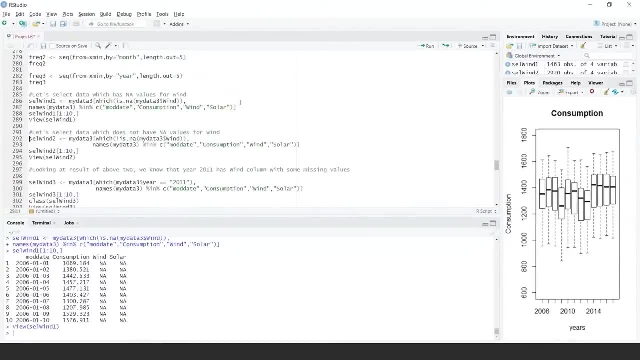 data in between where wind has some values. so we have found out NA values. now what we will do is we will select data which does not have NA values, so I will call it cell selected: wind. 2- I will again use my data. 3- I will say which. but now 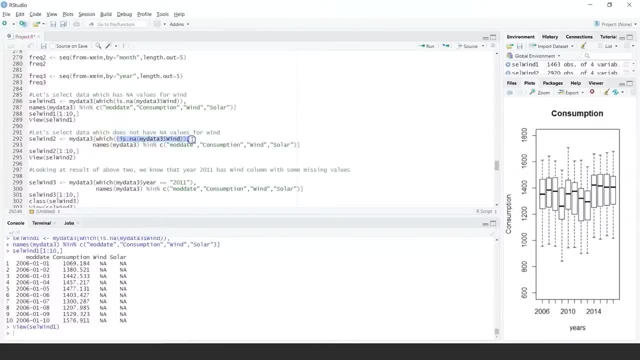 I am saying not NA from this column and I will select the data for the columns. so I am interested in looking at 10 records and this shows me not NA values. so no more missing values. so if I really look at this data, as I saw earlier, 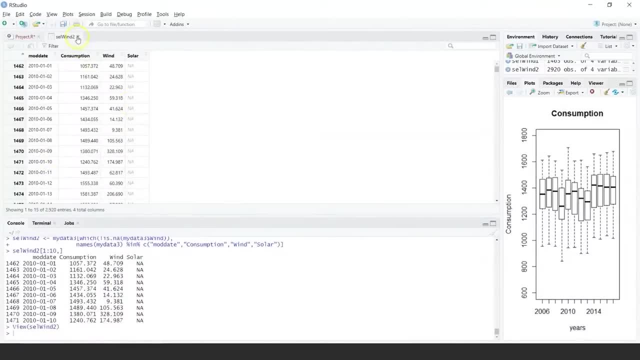 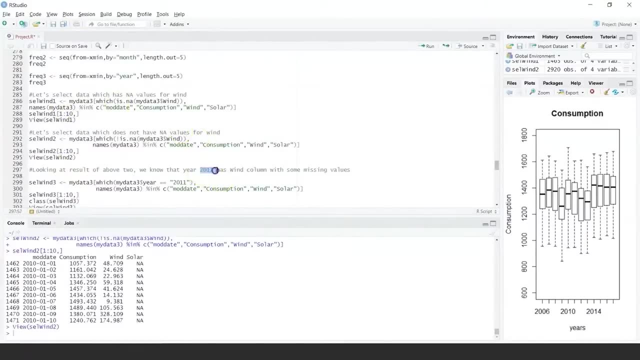 which has NA, and if I look at these values which are not NA for the wind column. so looking at these two result, we will know that in year 2011, wind column has some missing values. so let's focus on year 2011. so how do I? 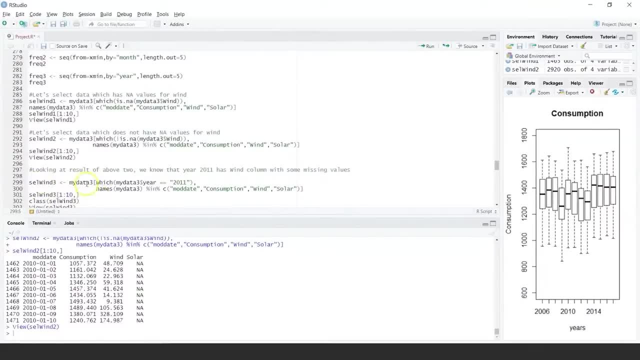 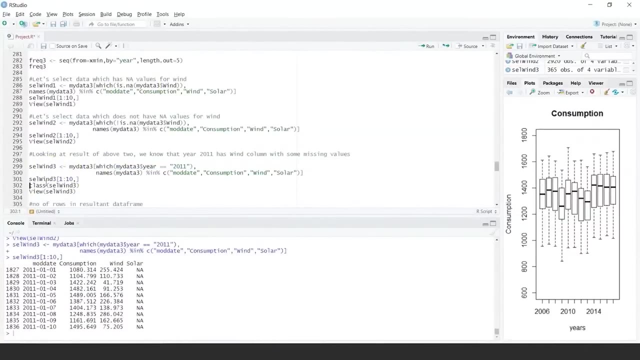 do that. let's call it a different variable. I will say my data 3. I will say here, when I say which, where we were saying NA, here I will say the year should have a value of 2011 and I want all these columns. let's look at the data here. 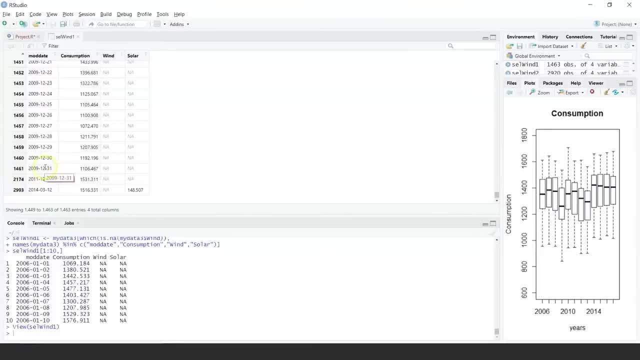 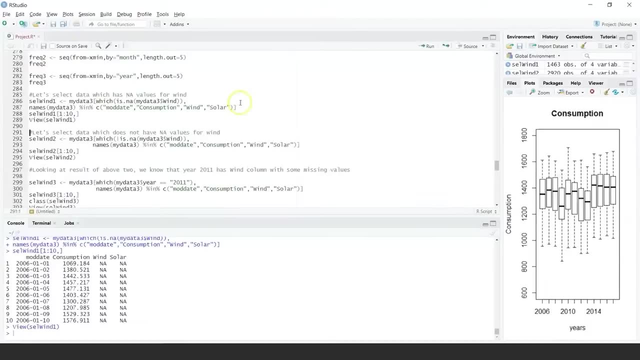 you have 1461 and then you have 2174, so there is a difference. so there is some data in between where wind has some values. so we have found out NA values. now what we will do is we will select data which does not have NA values. 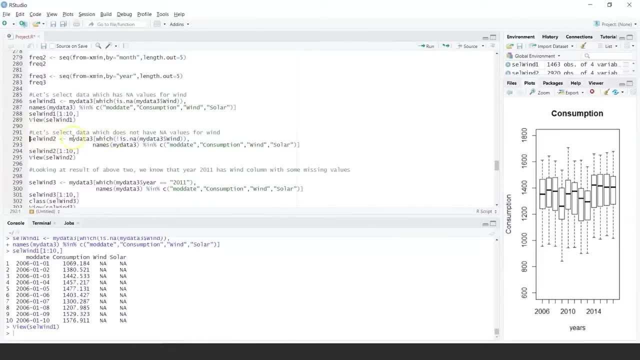 so i will call it cell selected wind. 2: i will again use my data. 3- i will say which, but now i am saying not NA from this column and i will select the data for the columns. so i am interested in looking at 10 records and this shows me. 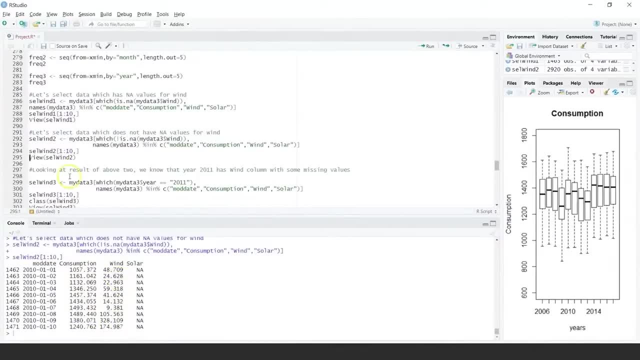 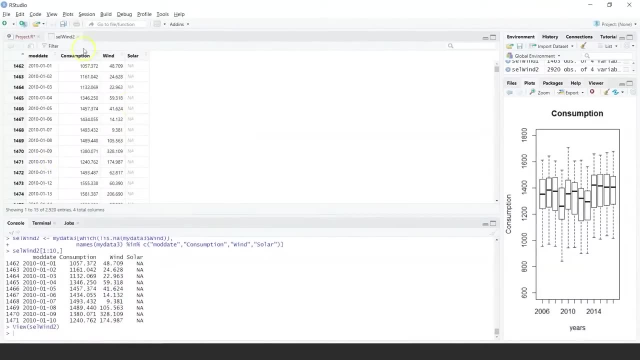 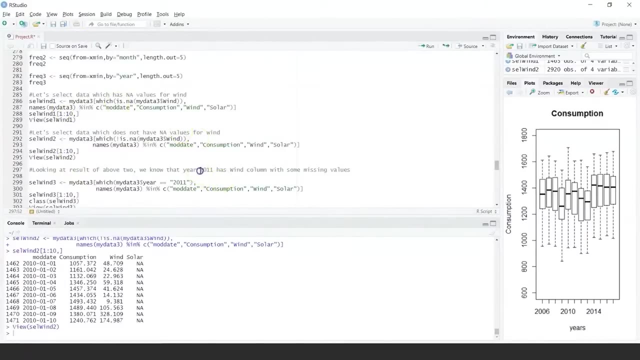 not NA values, so no more missing values. so if i really look at this data, as i saw earlier, which has NA, and if i look at these values which are not NA for the wind column, so looking at these two result, we will know that in year 2011. 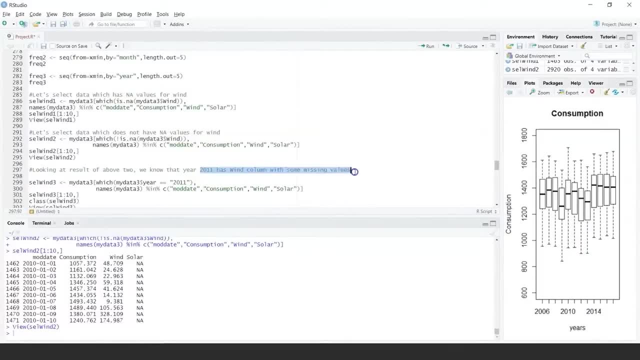 wind column has some missing values, so lets focus on year 2011. so how do i do that? lets call it a different variable. i will say my data 3, i will say here. when i say which, where we were saying NA, here i will say the year should have a value of 2011. 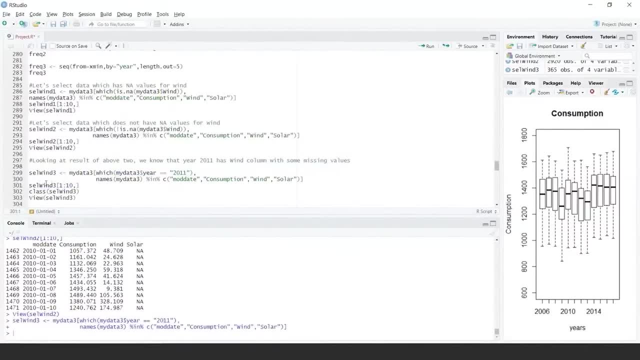 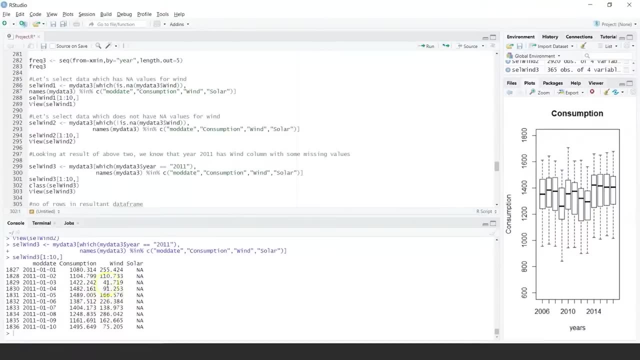 and i want all these columns. lets look at the data here, and this is showing me 2011, but we are not seeing all the values. so there are some values, but then there are some missing values, also for 2011, based on whatever analysis we have done. so lets look. 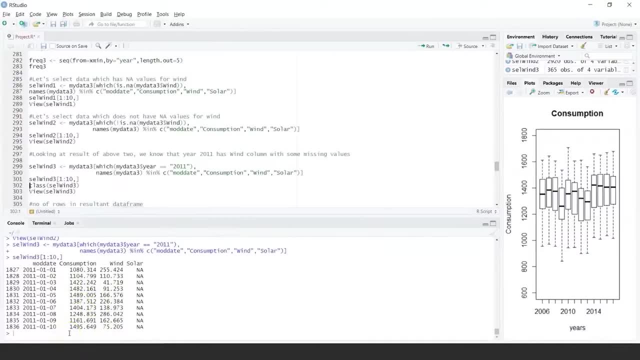 and this is showing me 2011, but we are not seeing all the values. so there are some values, but then there are some missing values, also for 2011, based on whatever analysis we have done. so let's look at the class of this. it is: 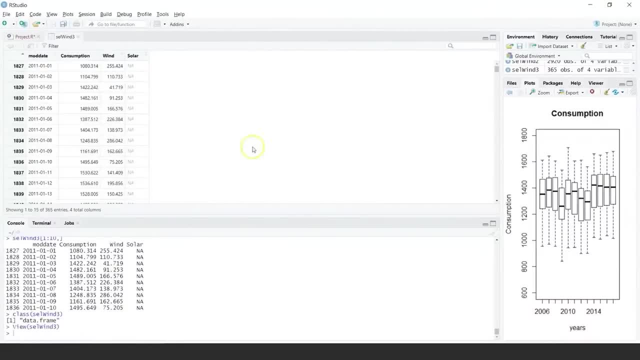 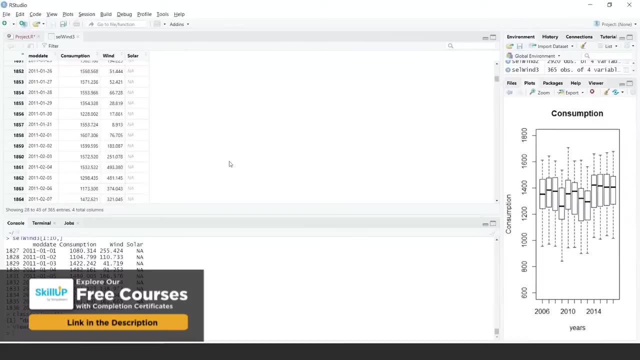 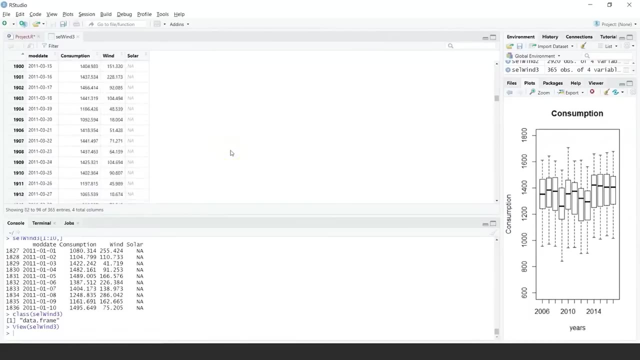 basically a data frame, do a view and this one will help me in finding out where are the NA values. so if you just scroll down, looking at all the data, let's search if wind column has a NA or a missing value and I will see if there is any missing value in. 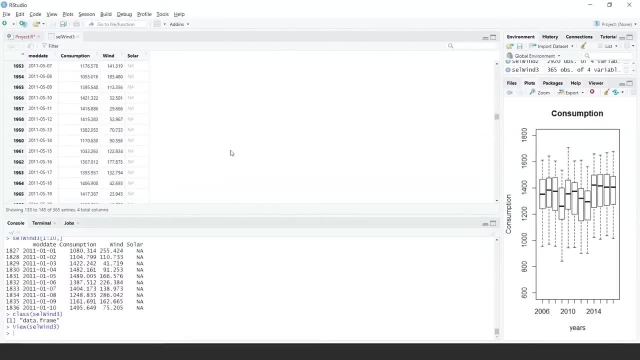 which column or which row it is for the wind column. so we have all the values which are existing. I could select and search for one specific value and I will show you how we can do that. so here let's scroll all the way down, so it's like you are. 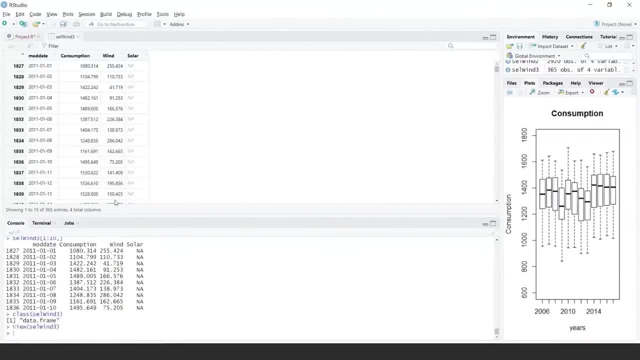 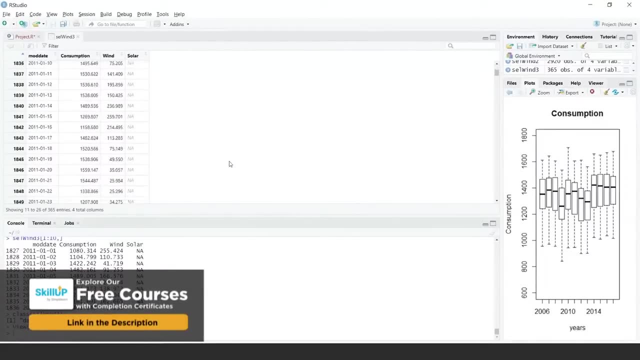 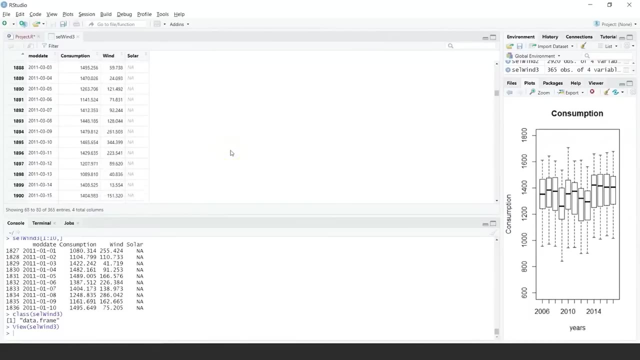 at the class of this- it is basically data frame- do a view and this one will help me in finding out where are the NA values. so if you just scroll down looking at all the data, lets search if wind column has a NA or a missing value and i will see if. 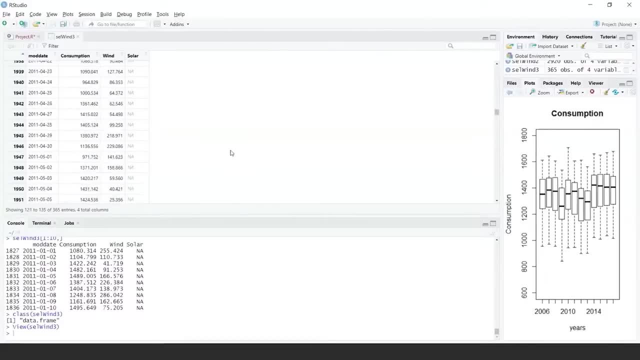 there is any missing value? in which column or which row it is for the wind column. so we have all the values which are existing. i could select and search for one specific value, and i will show you how we can do that. so here lets scroll all the way. 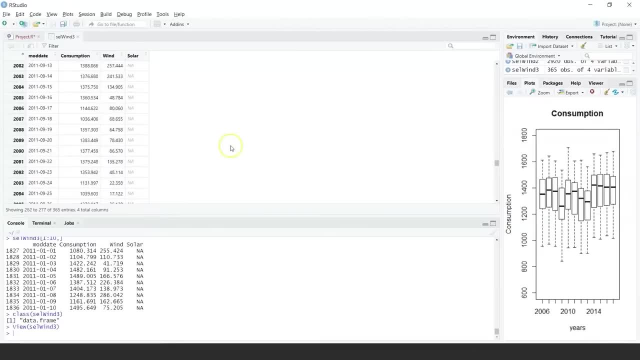 down. so its like you are exploring your data and seeing: is wind column having NA or missing value for a particular row? and lets scroll here and here you see there is a missing value for one particular row. so 13th December 2011 has wind value. 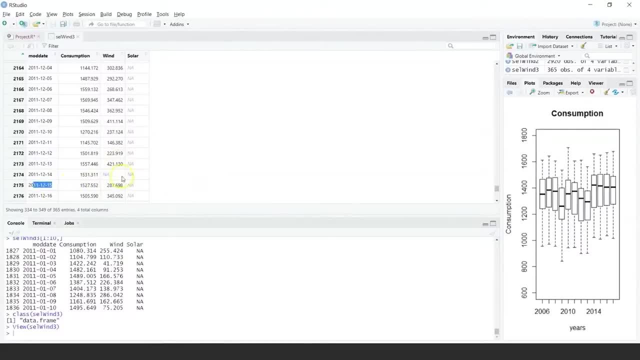 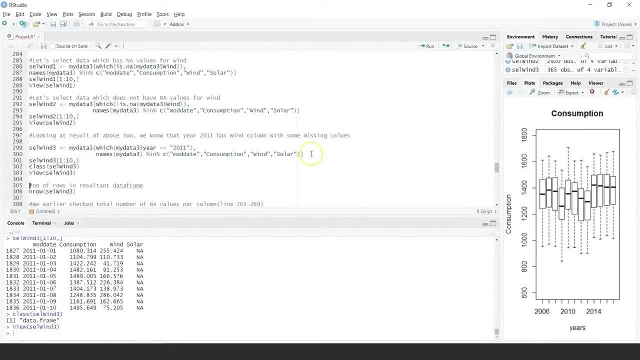 15th December has wind value, but your 14th December does not have right. similarly, we can search. so there was only one entry which was missing. now that could be for some reason, might be it was not calculated, might be it was not tabulated. so we have a missing value and that. 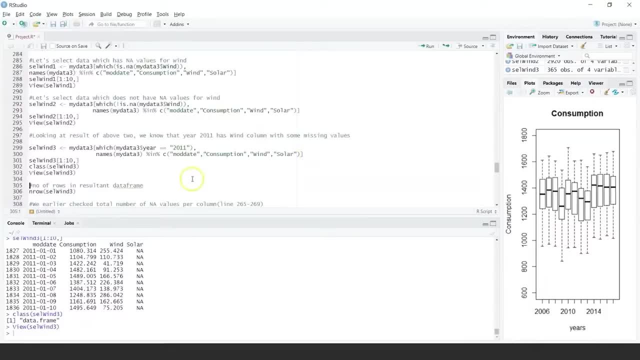 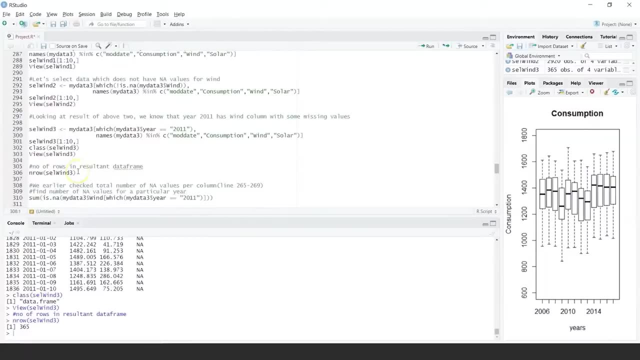 can effect my plotting, that can effect my analysis. so lets look at the number of rows in this, which will tell me how many rows we have for 2011. so it tells me 365. so that is basically the number of days in a year. now we will find. 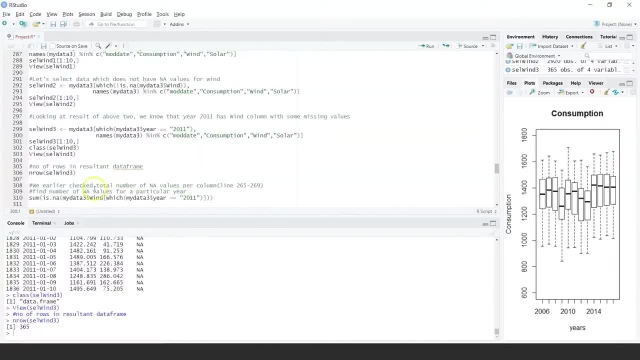 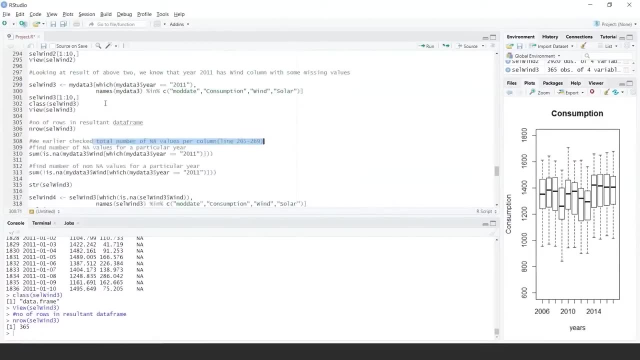 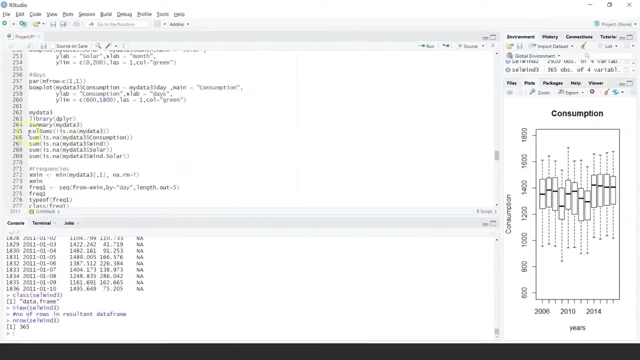 out if there were NA values. so we earlier checked total number of NA values per column. that is, in your row number 265 to 269. we can see here 265 to 269. so this is where we were seeing. are there any NA values? right, so lets go back. 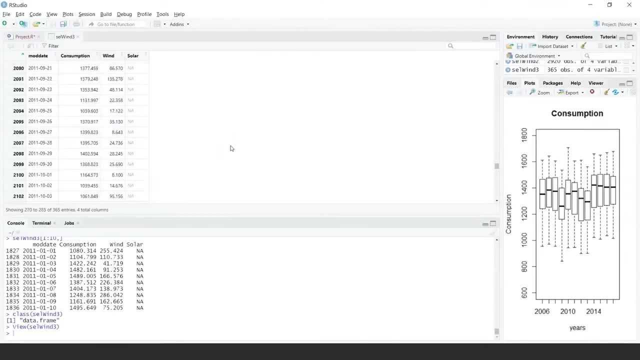 exploring your data and seeing: is wind column having NA or missing value for a particular row? and let's scroll here and here you see there is a missing value for one particular row. so 13th December 2011 has wind value. 15th December has wind value, but 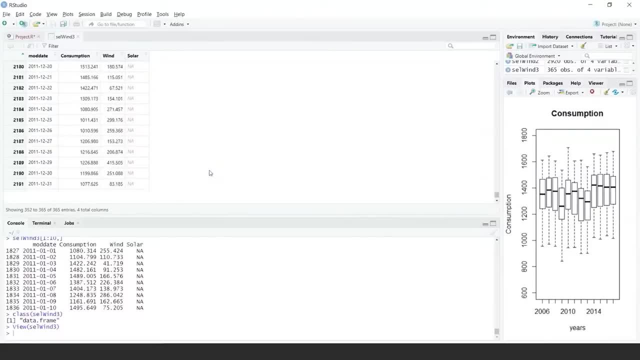 your 14th December does not have right. similarly, we can search. so there was only one entry which was missing. now that could be for some reason, might be it was not calculated, might be it was not tabulated. so we have a missing value and that can effect my 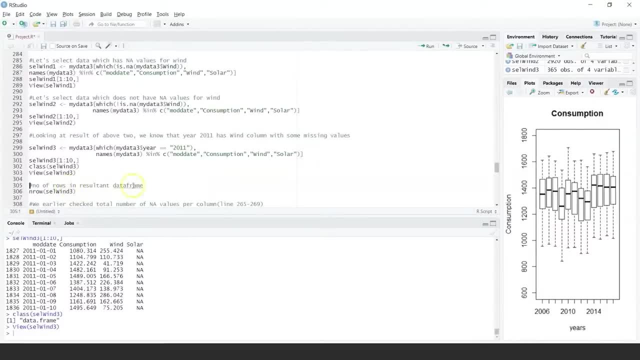 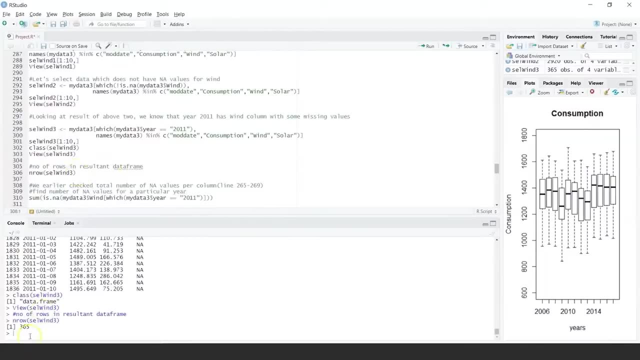 plotting that can effect my analysis. so let's look at the number of rows in this, which will tell me how many rows we have for 2011. so it tells me 365. so that is basically the number of days in a year. now we will find out if. 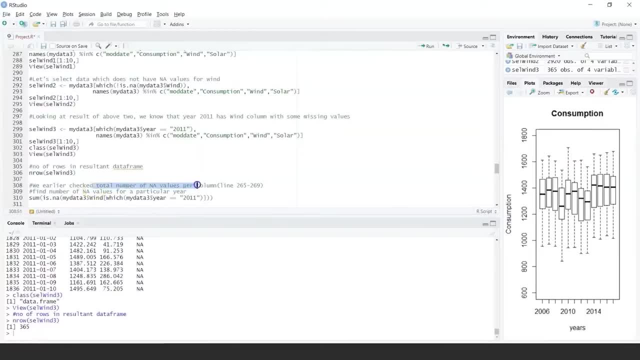 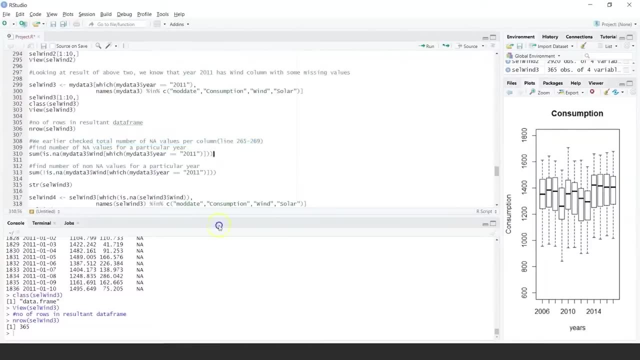 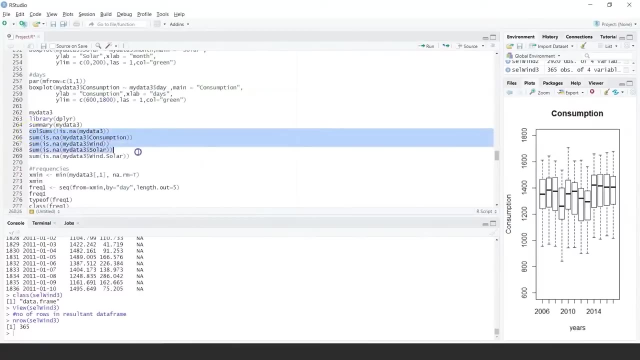 there were NA values. so we earlier checked total number of NA values per column. that is, in your row number 265 to 269. we can see here 265 to 269. so this is where we were seeing. are there any NA values? right? so let's go back here. 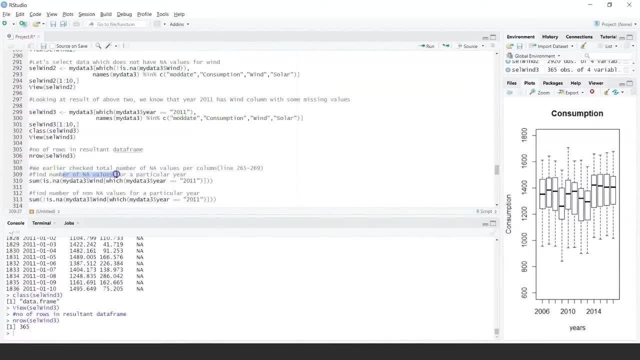 and we want to find out the number of NA values for a particular year. how do I do it? so I can just do a sum I will say is NA. now I am interested in my data 3 wind column and I am saying my year has to be 2011, but I am finding out. 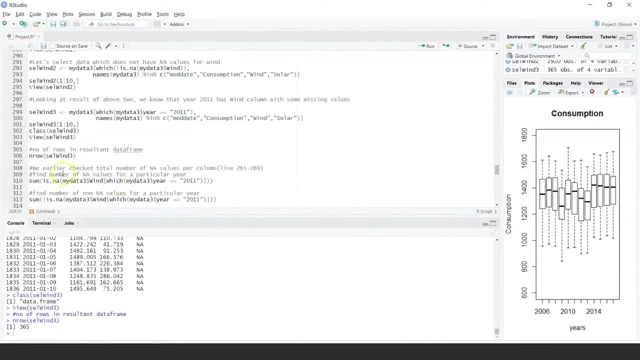 here and we want to find out the number of NA values for a particular year. how do i do it? so i can just do a sum i will say is NA. now i am interested in my data, 3 wind column, and i am saying my year has to be. 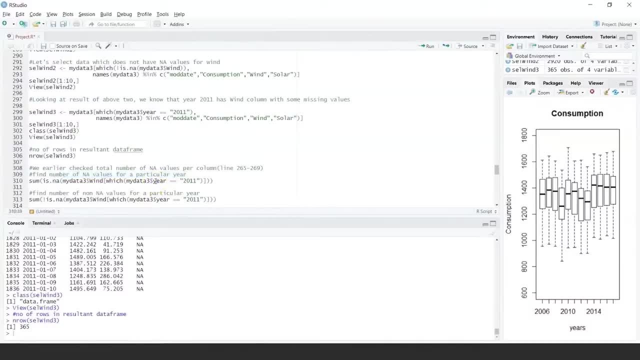 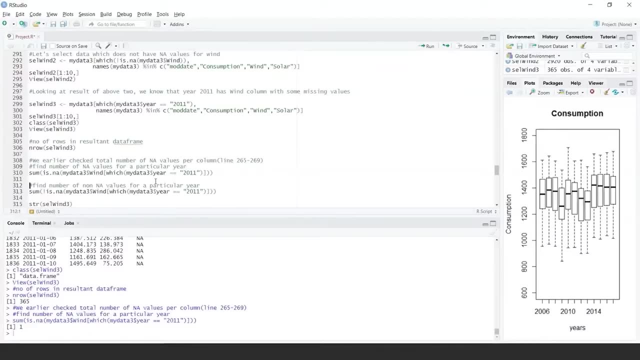 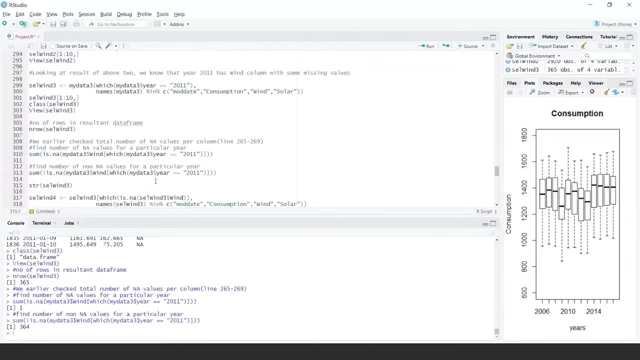 2011, but i am finding out the NA values. so lets do this and it tells me 1, and thats right. thats what we saw when we did a view. lets see how many non NA values you have, and that is 364, so that basically satisfies my logic, so its. 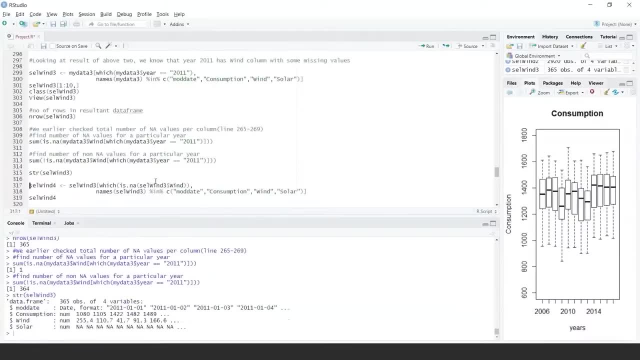 364 plus 1 missing, so there are 365. lets look at the structure of this. it tells me you have modified date and date format. you have consumption, wind and solar. now lets create a variable, selected wind 4, i will say wind 3, that is. 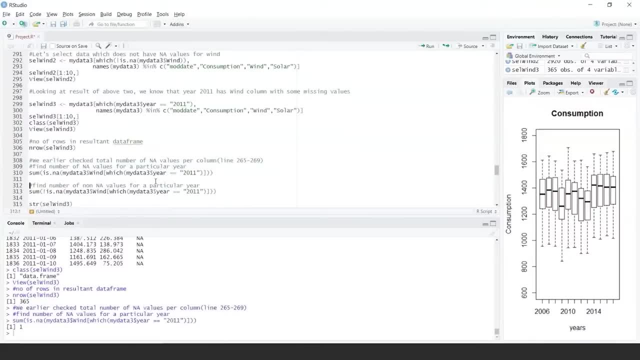 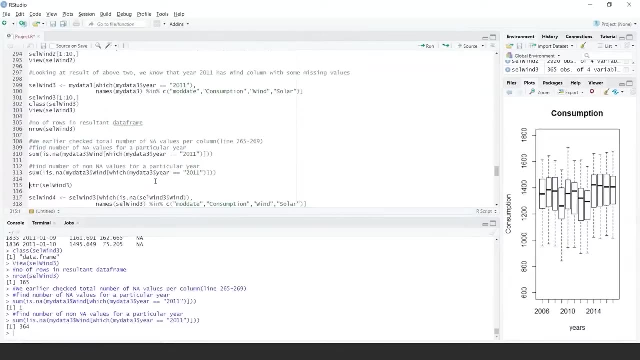 the NA values. so let's do this, and it tells me 1, and that's right. that's what we saw when we did a view. let's see how many non NA values you have, and that is 364. so that basically satisfies my logic. so 364 plus 1 missing. so 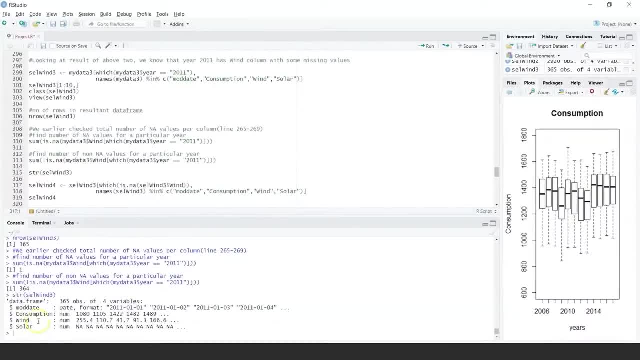 there are 365. let's look at the structure of this. it tells me you have modified date and date format. you have consumption, wind and solar. now let's create a variable selected wind 4, I will say wind 3. that is which was having all my 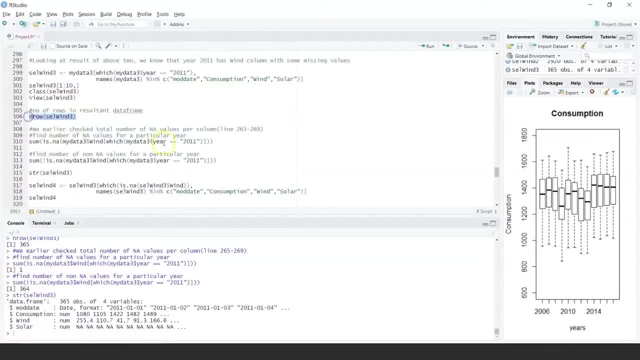 which was having all my NA and non NA values for 2011. i will say: lets find out the NA value, because i am interested in finding out that particular row. so i am saying: find out where the value is NA and i want all the columns. lets. 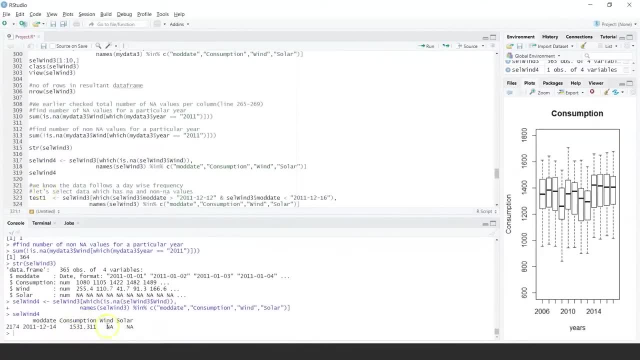 look at this one, and this is my specific row, which has a NA value. now we know that data follows a day wise frequency, which we have clearly seen now, lets select data which has NA and non NA values. so lets say, lets call it test1. i will use wind 3, which has 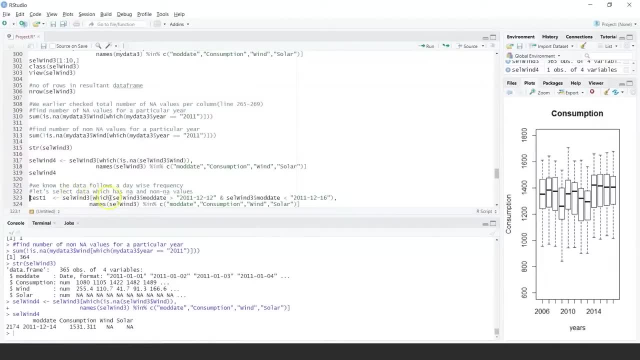 NA and non NA values. but now i will say i want the modified date, which should be greater than 12 12 2001. now, remember we had, when we were doing, a view. we saw that one particular day or what we see here. 14th, 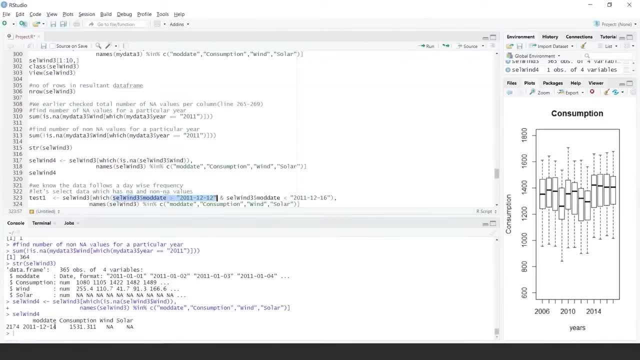 of December. there is no date, so i will select a subset of data which includes this NA and non NA, that is, might be i can take 15th of December and 15th of December, so lets start from 12- 12, so the date should be greater. 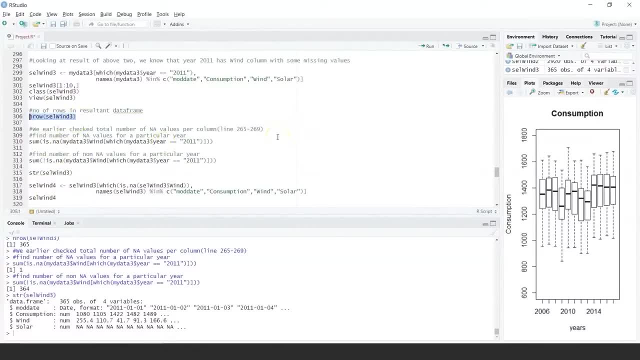 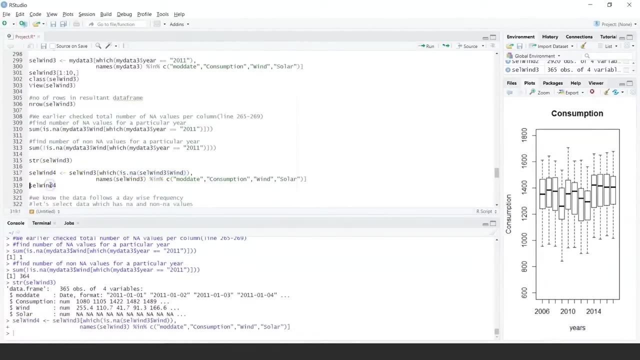 NA and non NA values for 2011. I will say: let's find out the NA value because I am interested in finding out that particular row. so I am saying: find out where the value is NA and I want all the columns. let's look at this one and this. 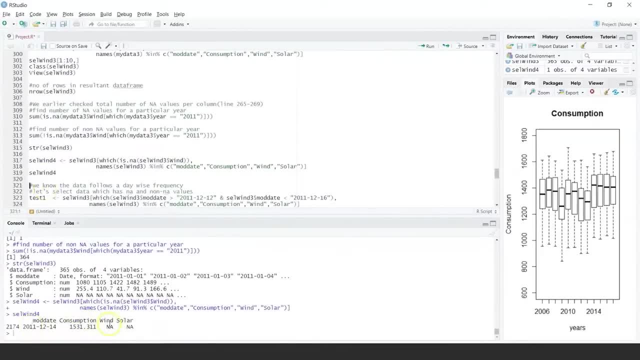 is my specific row which has a NA value. now we know that data follows a day wise frequency, which we have clearly seen. now let's select data which has NA and non NA values. so let's say, let's call it test 1. I will use wind 3. 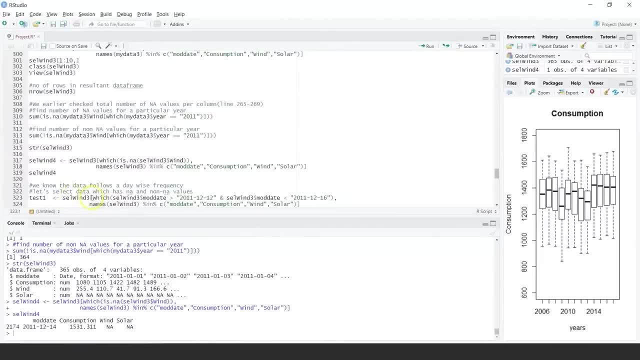 which has NA and non NA values. but now I will say I want the modified date, which should be greater than 12 12 2001. now, remember, we had, when we were doing, a view. we saw that one particular day, or what we see here, is a month of December. 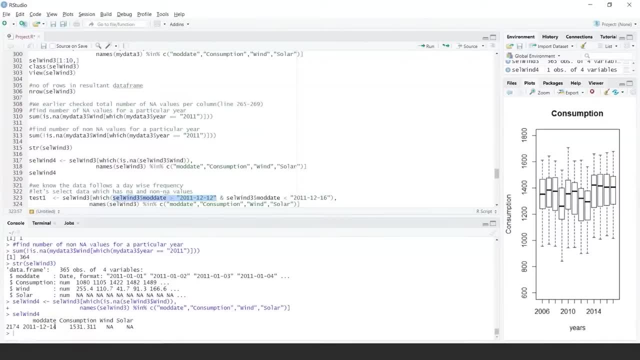 there is no date, so I will select a subset of data which includes this NA and non NA, that is might be. I can take 13th of December and 15th of December, so let's start from 12- 12, so the date should be greater than 12. 12 that means 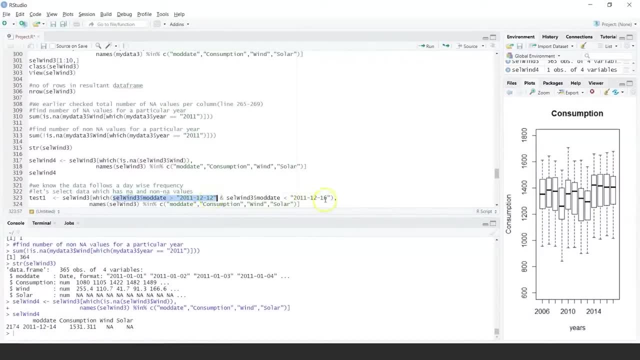 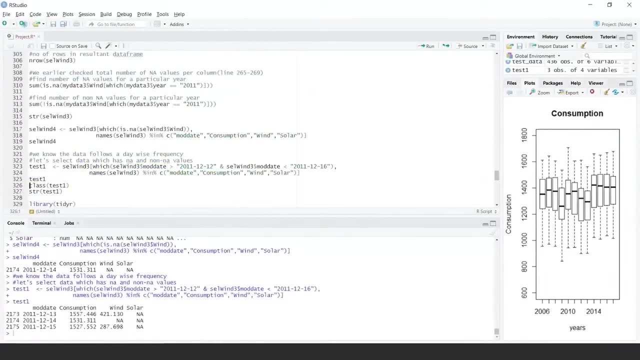 than 12. 12, that means 13th, and it should be less than 16. so that is 15th and the columns right. so now we have some data. lets look at this. so i have a. i have selected a subset of data. i could have done this using subset. 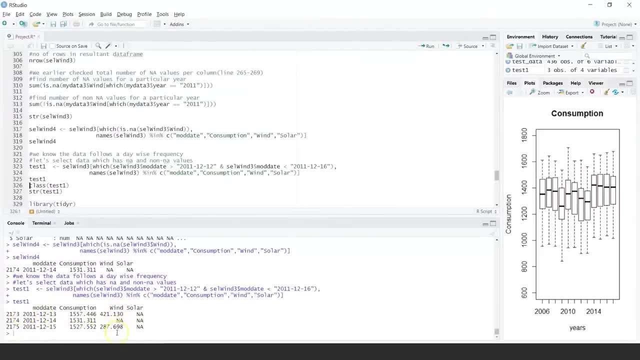 also. so i have NA and non NA values. now why are we doing this? so sometimes you might have some data for a particular column and you may want to find out if there are any missing values. might be you want to fill them up or replace them with something. 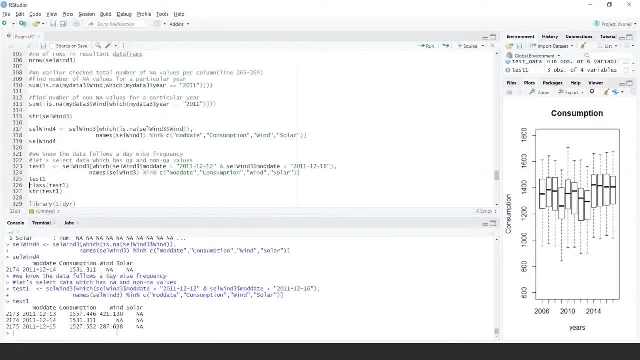 so that is usually useful when you are doing a trend detection. so say, for example, you have data for every month and might be in one of the months you have missed, or might be you have data for every year, collected monthly, and then in one of the years for couple of months you don't have. 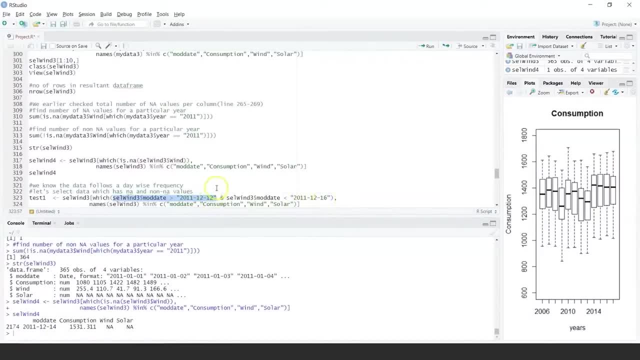 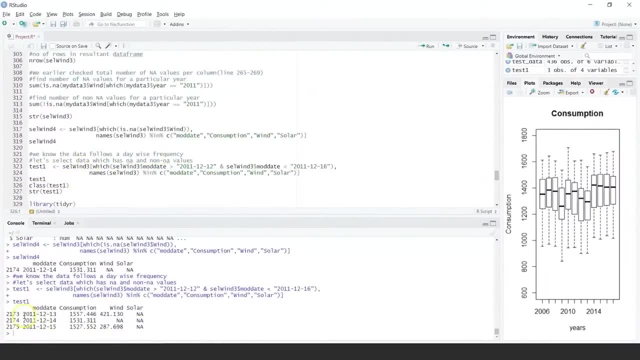 13th and it should be less than 16. so that is 15th and the columns right. so now we have some data. let's look at this. so I have a. I have selected subset of data. I could have done this using subset also, so I have. 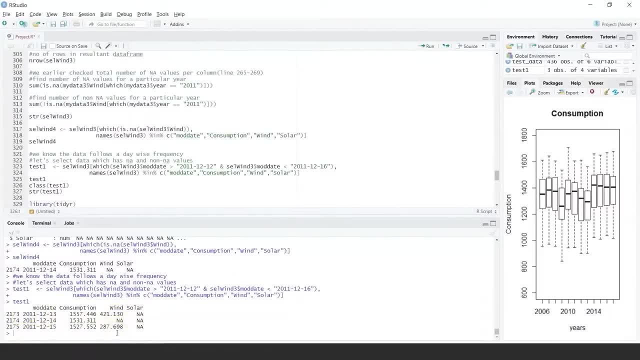 NA and non NA values. now why are we doing this? so sometimes you might have some data for a particular column and you may want to find out if there are any missing values might be you want to fill them up or replace them with something, so that is usually. 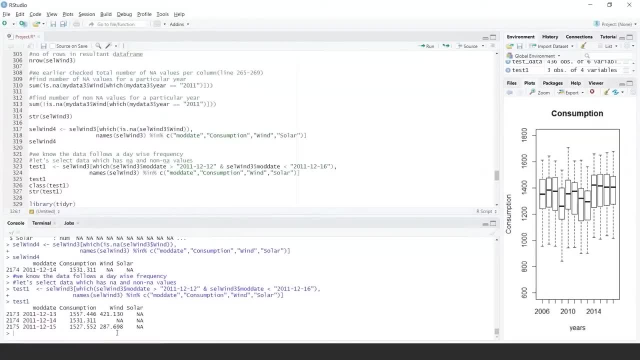 useful when you are doing a trend detection. so say, for example, you have data for every month and might be in one of the months you have missed, or might be you have data for every year, collected monthly, and then in one of the years, for couple of months you don't. 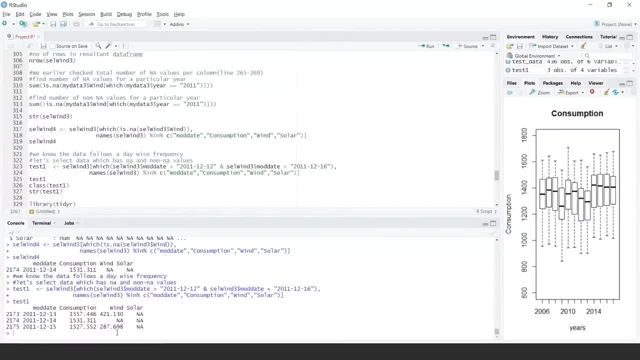 have the data, like I can say 2016. I have data for all 12 months 2017, all 12 months 2018 might be. I don't have data for March and June 2019. I don't have data for same months, so I can. 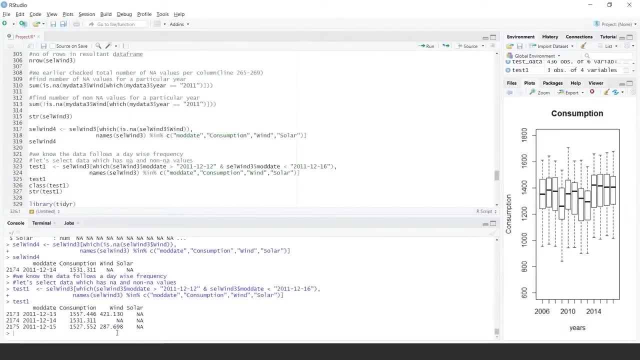 the data, like i can say 2016. i have data for all 12 months 2017, all 12 months 2018 might be. i don't have data for march and june 2019. i don't have data for same months, so i can forward. 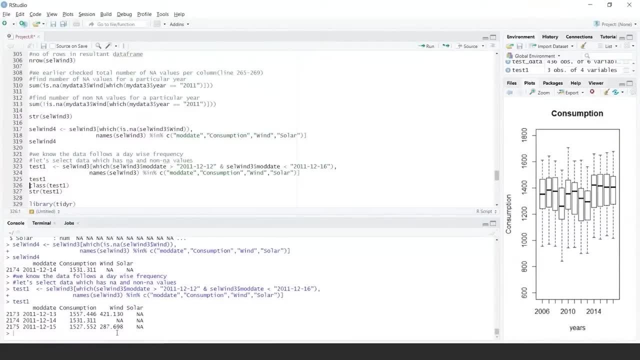 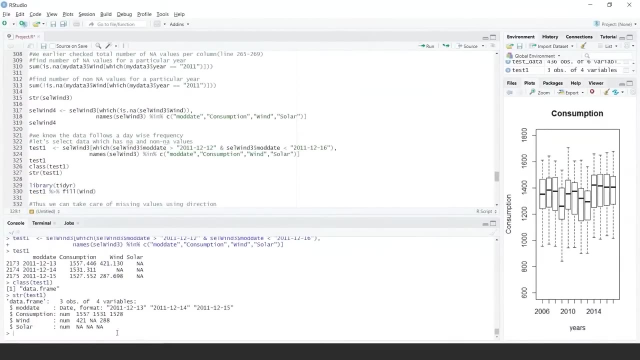 fill or backward fill them using the previous years, same month data, so we can do that. so here i have test data where i have extracted a subset of data. i can look at the class of this. it is a data frame structure of this. it has the columns. now let's 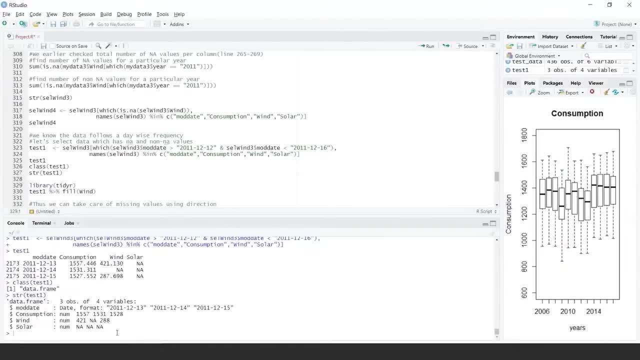 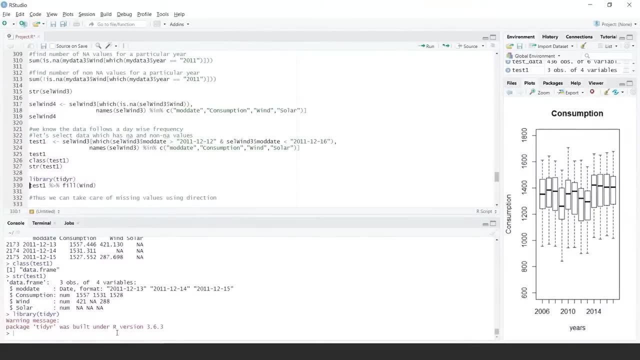 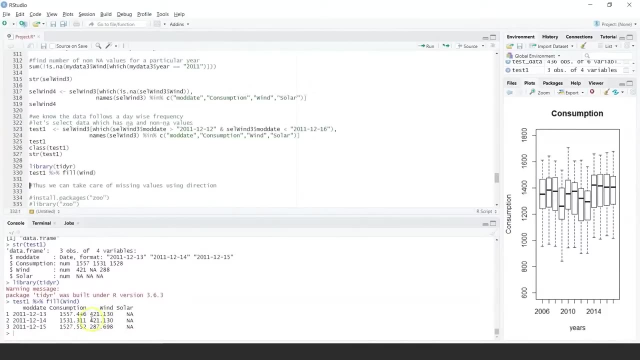 use the library and function and use the tidy r package and what we will do is we will fill it up. so i will use test one. i will fill the wind column, which has a missing value now. once you do this, if you notice it has done a forward fill. 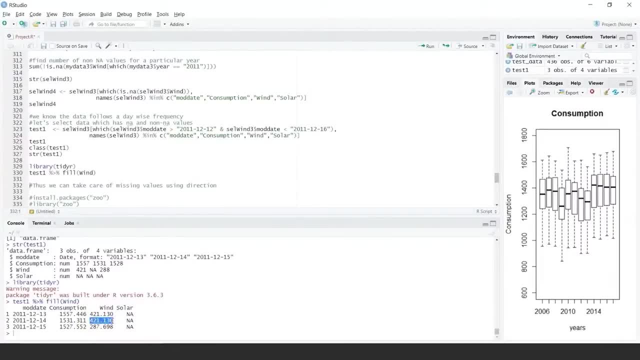 so it has taken the previous value and it has just filled up that, so you can fill up the data using different directions, such as up and down, left and right and so on, so we can take care of missing values in our frequency data, which allows us to basically 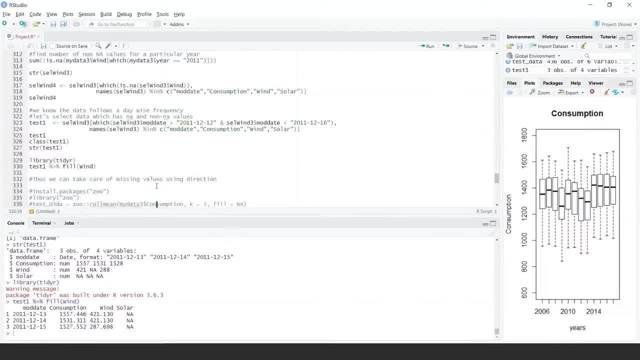 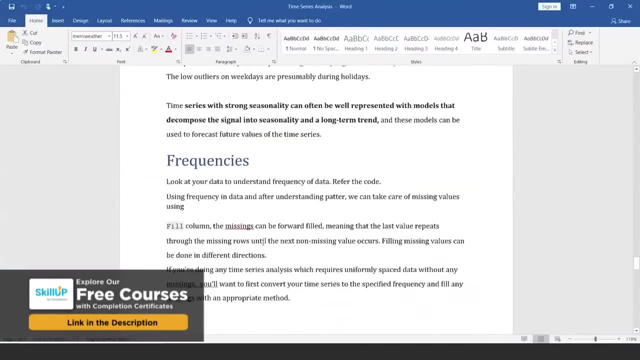 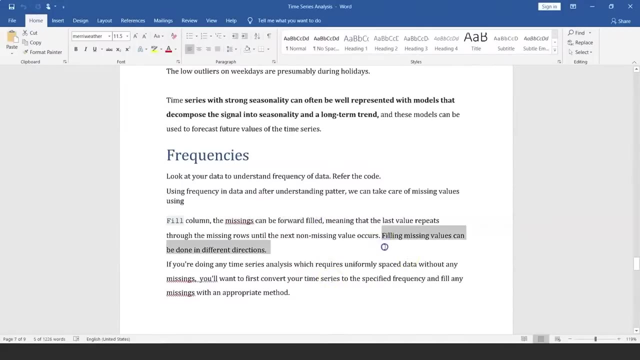 analyze the data in a better way. now here we will want to also look at some more data. so this is to deal with frequencies of fill column, wherein you can take care of missing values forward fill, so filling values can be done in different directions, as i said. 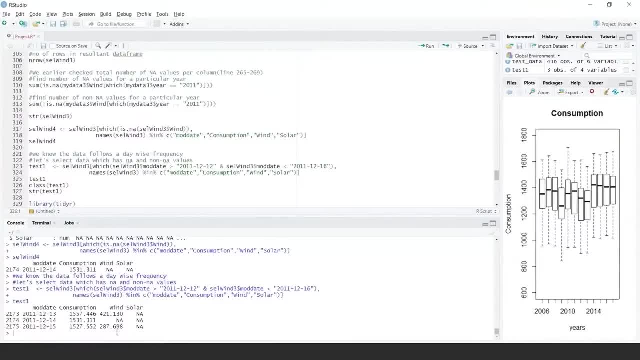 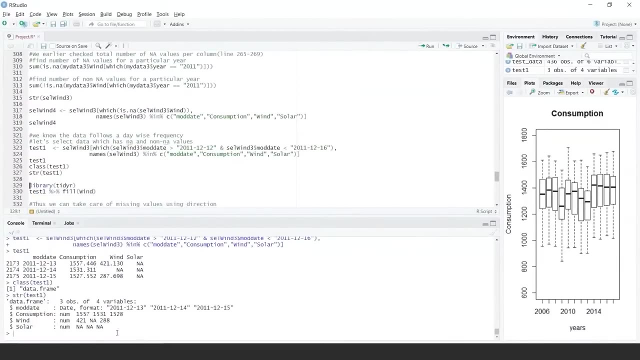 forward fill or backward fill them using the previous years same month data. so we can do that. so here I have test data where I have extracted a subset of data. I can look at the class of this. it is a data frame structure of this. it has the columns now. 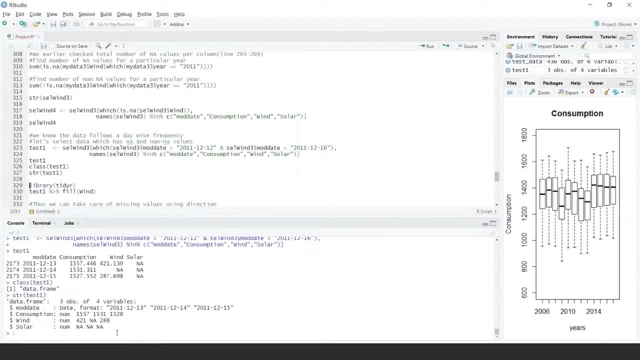 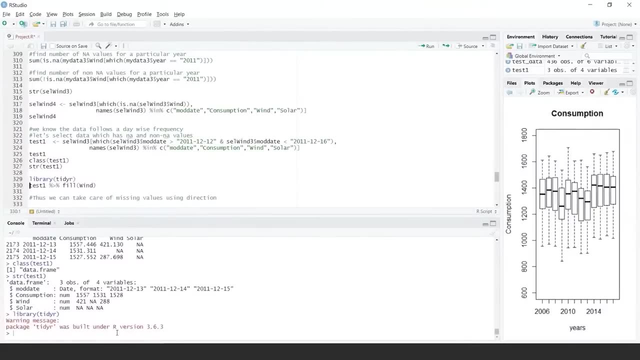 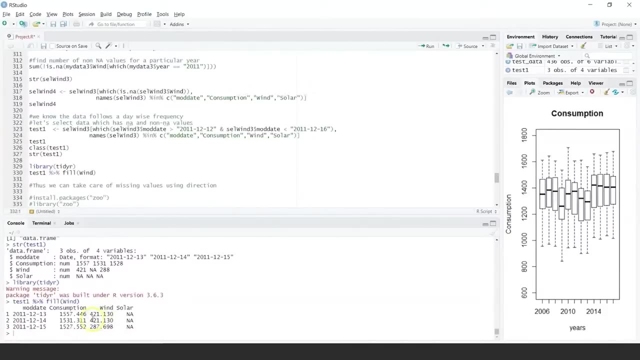 let's use the library and function and use the tidy R package and what we will do is we will fill it up. so I will use test one. I will fill the wind column which has a missing value. now, once you do this, if you notice it has done a forward. 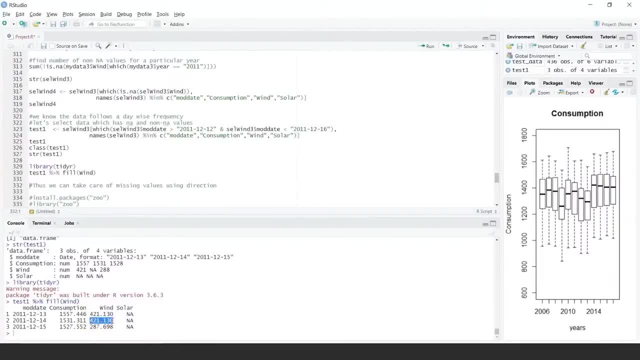 fill. so it has taken the previous value and it has just filled up that, so you can fill up the data using different directions, such as up and down, left and right and so on, so we can take care of missing values in our frequency data, which allows us to. 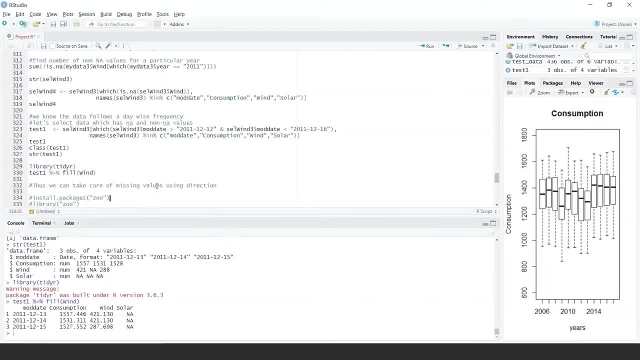 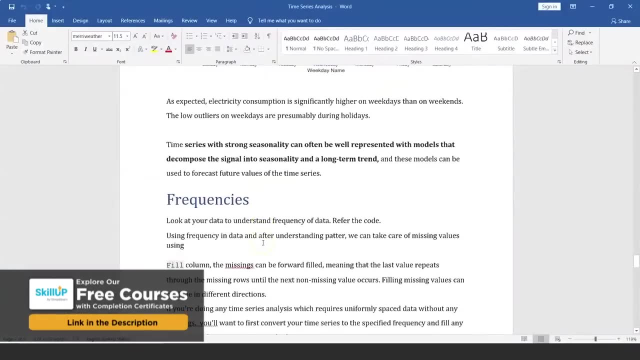 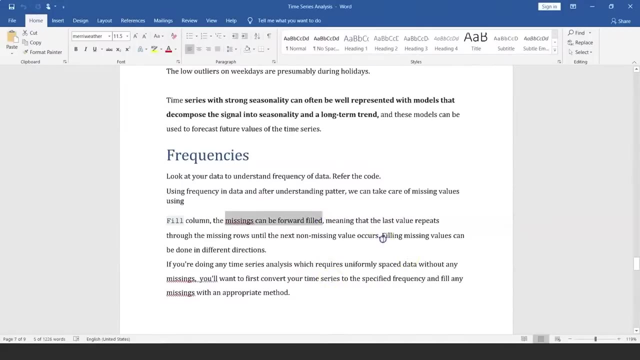 basically analyze the data in a better way. now here we will want to also look at some more data. so this is to deal with frequencies of fill column, wherein you can take care of missing values forward filled, so filling values can be done in different directions, as I 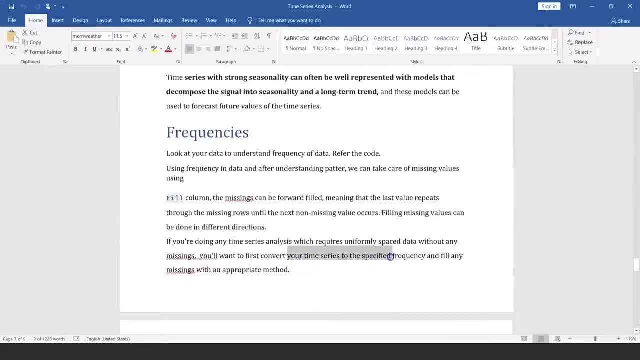 said, and you may want to first convert your time series to specified frequency. if your data does not have a frequency- but we had now- if you do not have a frequency, might be- you can convert it into a frequency such as weekly, daily, monthly, as I showed you. 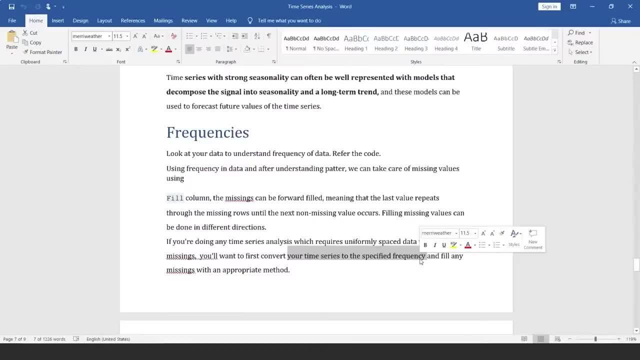 and then basically you can do a forward fill for the values. so, for example, if I have my data, I can break it down into weekly and then look at the values and if there are any values missing for weekly data I can use a forward fill. so that can take. 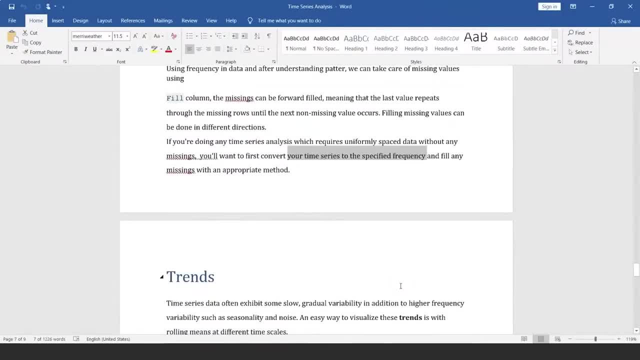 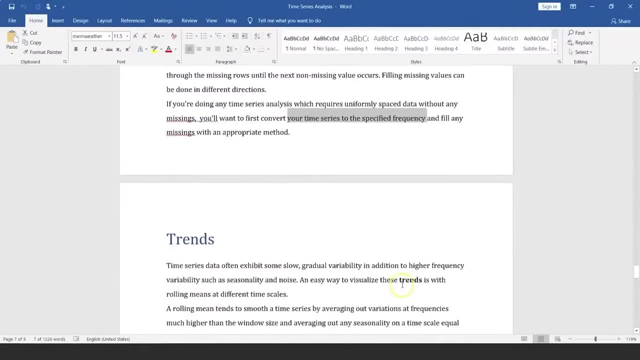 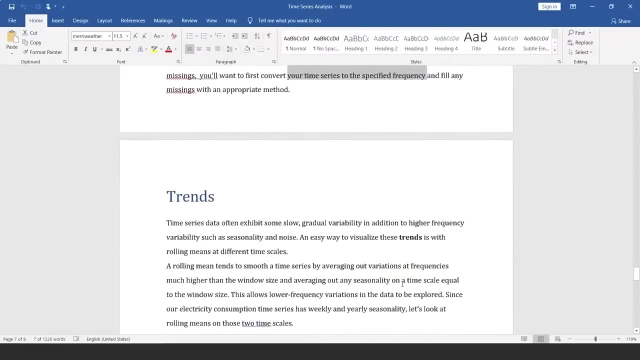 care of my frequency data. then let's look at the trends of the data, which is the last part of this project. so basically, let's look at the trend. so when you say trend, what does that mean? so in time series data, you always have some kind of trend. 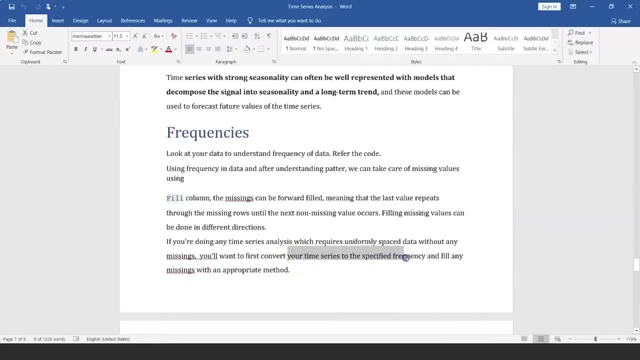 and you may want to first convert your time series to specified frequency. if your data does not have a frequency- but we had now, if you do not have a frequency, might be- you can convert it into a frequency such as weekly, daily, monthly, as i showed you, and then 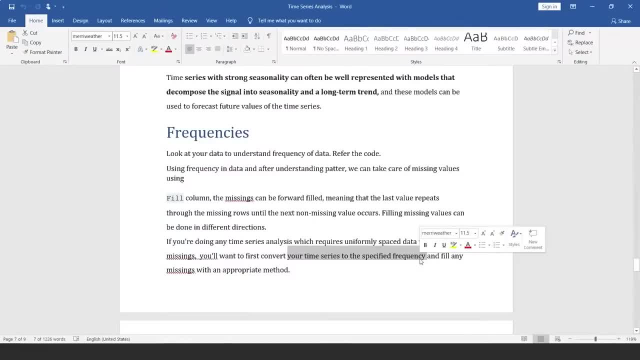 basically you can do a forward fill for the values. so for example, if i have my data i can break it down into weekly and then look at the values and if there are any values missing for weekly data i can use a forward fill. so that can take care of. 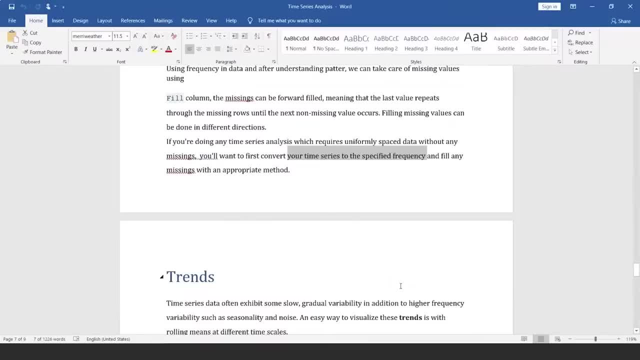 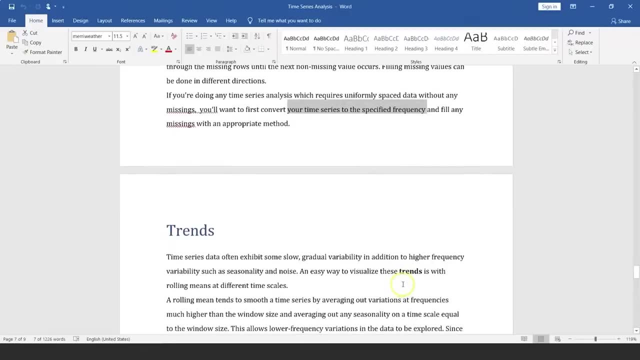 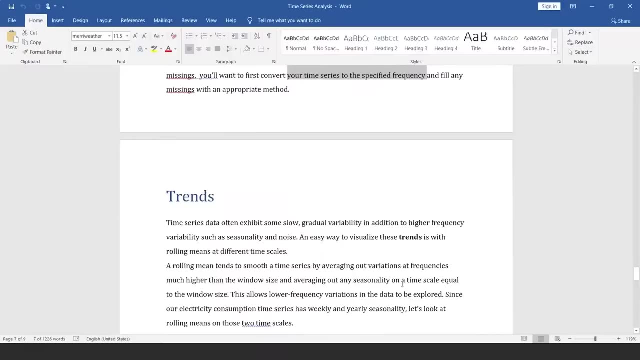 my frequency data. then lets look at the trends of the data, which is the last part of this project. so basically, lets look at the trend. so when you say trend, what does that mean? so in time series data you always have some kind of trend, so that will exhibit some slow. 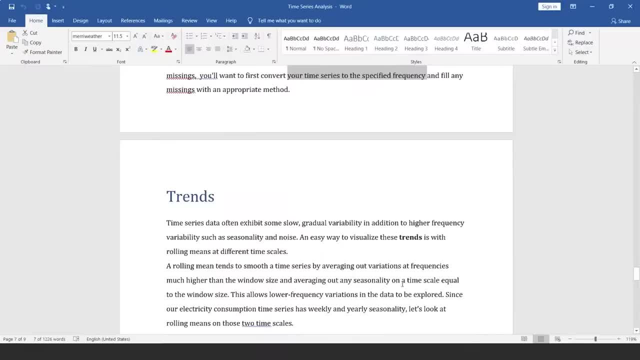 so that will exhibit some slow, gradual variability, in addition to higher frequency variability such as seasonality and noise. now, to visualize these trends, what we do is we use what we call as rolling means, so we know how our data is spread over year or month or day. 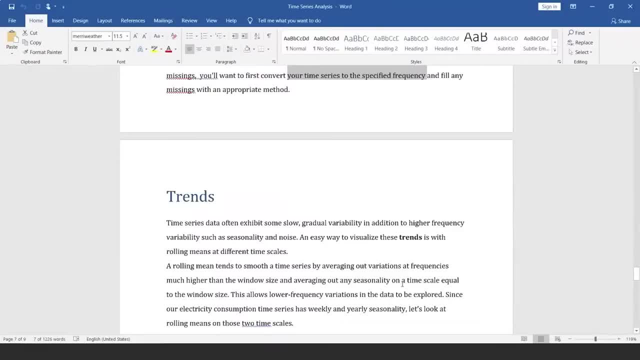 but how about looking at a rolling average and see what is the difference? so a rolling average, as seen, will tend to smooth a time series by averaging out the variations and frequencies. so this can be higher than the window size, so there is something called as windowing. 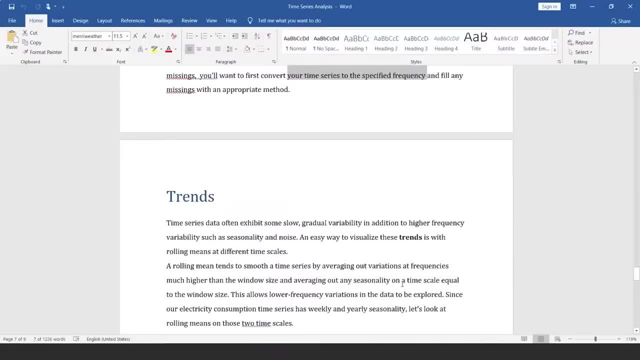 where you can choose a set of time frame. you can also average out any seasonality on a time scale equal to window size. so this will allow you to look at lower frequency variation in the data. so when we are looking at electricity consumption time series, we already 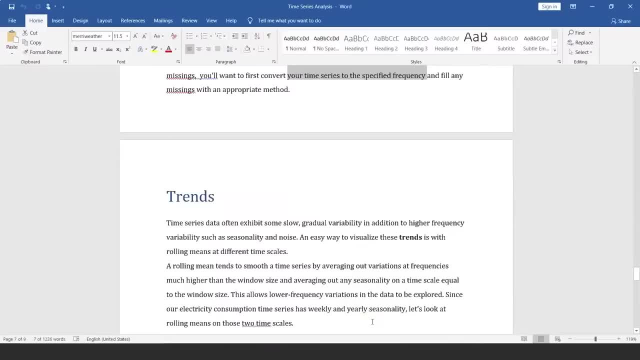 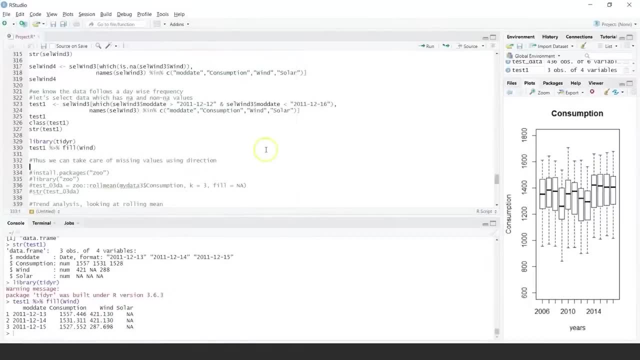 saw, there is a weekly pattern, there is a yearly seasonality, which we saw using box plots, so we can also look at the rolling means of the time scales. how do we do that? so for this you can use some package like zoo, and then you can basically use. 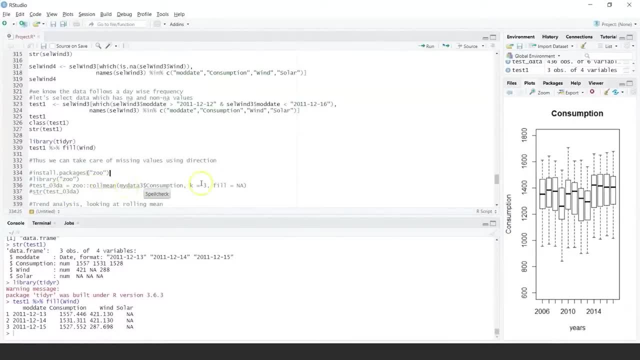 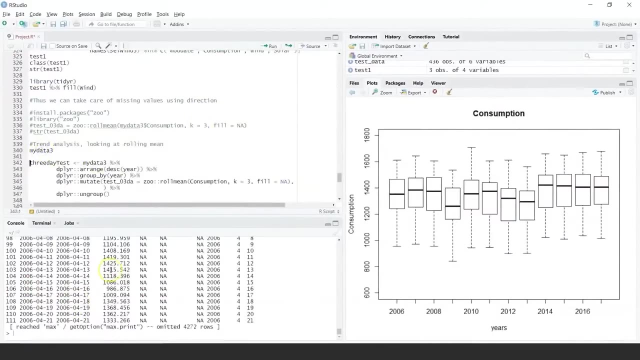 a rolling mean using the zoo package and you can say what is the frequency with which you want to calculate the rolling mean. now, how do we do this? let's look at this data. so here I am going to my look at my data 3, which we have been using so far. 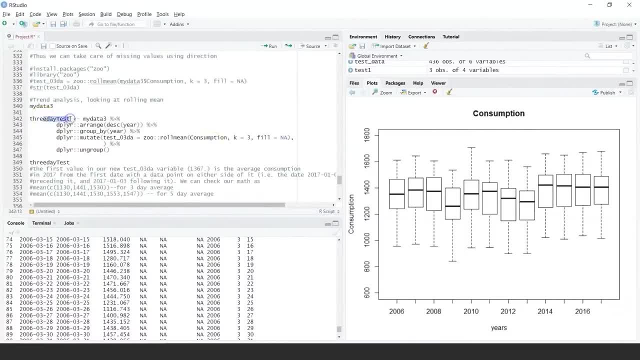 now let's call it a 3 day test. you can give it any name. I am going to use my data 3, I am using the pipe in function. now I will use dplyr and I will arrange the data descending in year. now you can always break it down step by step. 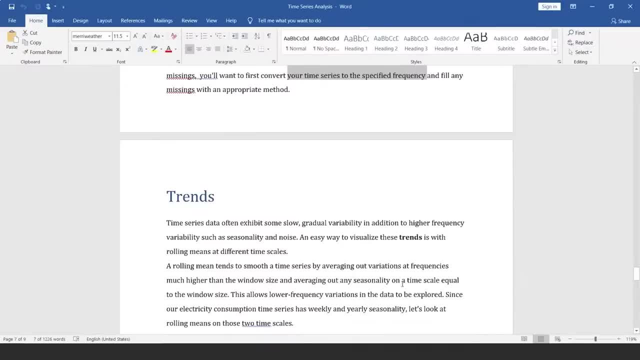 gradual variability, in addition to higher frequency variability such as seasonality and noise. now, to visualize these trends, what we do is we use what we call as rolling means, so we know how our data is spread over year or month or day. but how about looking at a rolling? 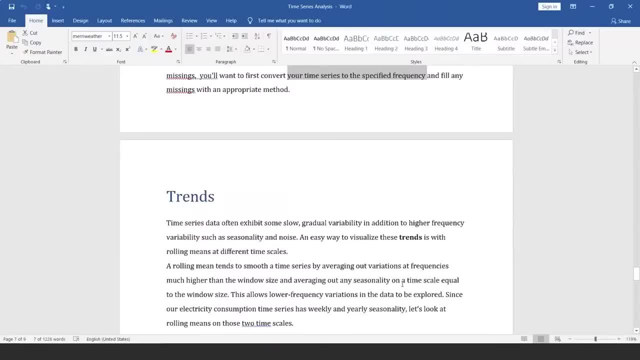 average and see what is the difference. so a rolling mean will tend to smooth a time series by averaging out the variations and frequencies, so this can be higher than the window size. so there is something called as windowing, where you can choose a set of time frame. 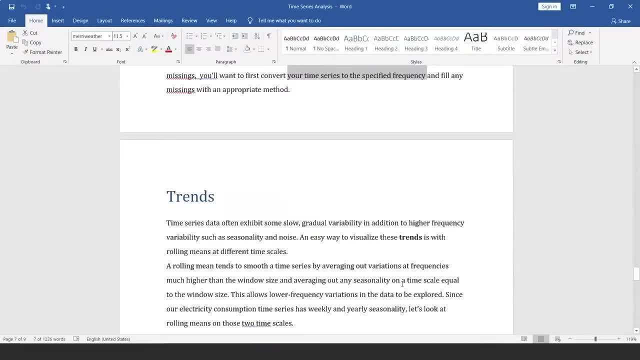 you can also average out any seasonality on a time scale equal to window size. so this will allow you to look at lower frequency variation in the data. so when we are looking at electricity consumption time series, we already saw there is a weekly pattern, there is a 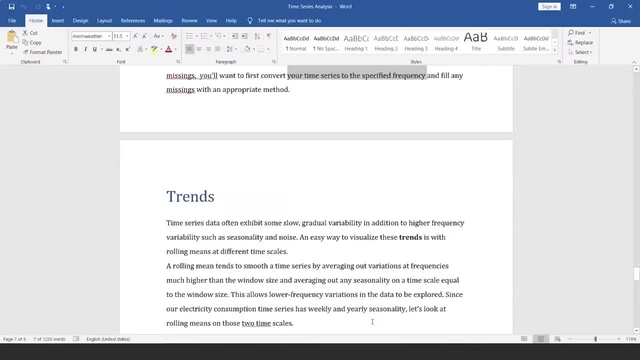 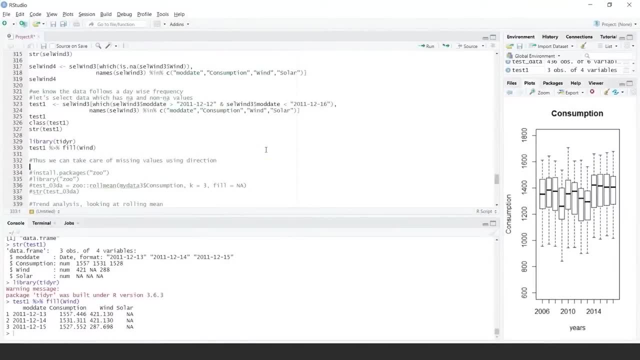 yearly seasonality, which we saw using box plots, so we can also look at the rolling means of the time scales. so how do we do that? so for this you can use some package like zoo, and then you can basically use a rolling mean using this zoo package and you can say: 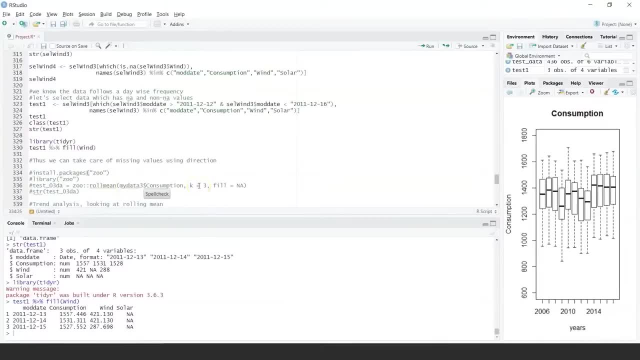 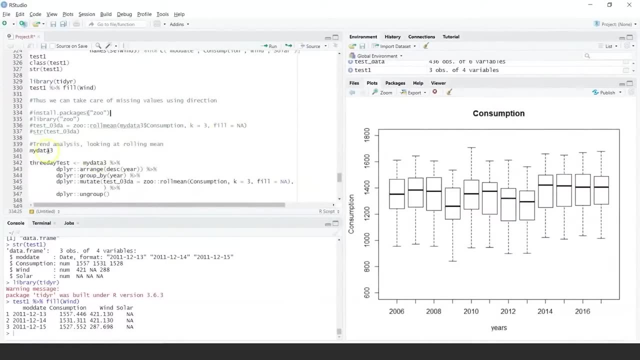 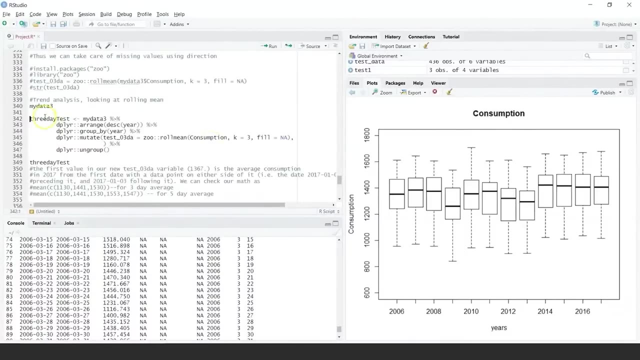 what is the frequency with which you want to calculate the rolling mean? now, how do we do this? let's look at this data. so here I am going to look at my data 3, which we have been using so far. now, let's call it a 3 day. 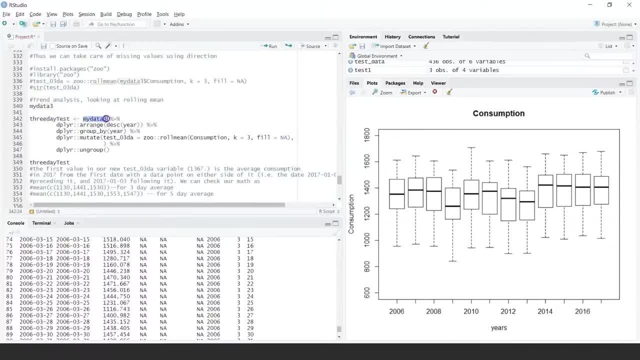 list. you can give it any name. I am going to use my data 3. I am using the pipe in function. now I will use dplyr and I will arrange the data descending in year. now you can always break it down step by step and you 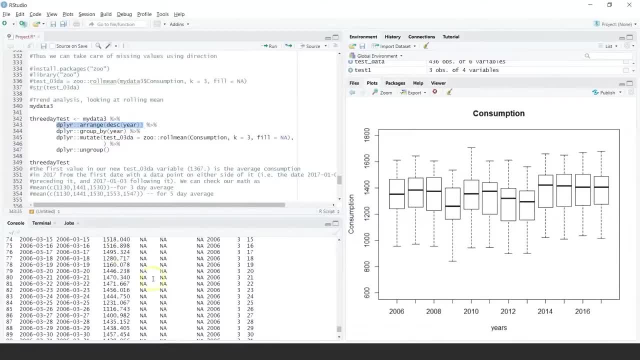 can see the result of this. so I am going to arrange this data in descending order of year, so obviously my last one, 2017 or 2018, will be on the top. you want to group the data by year, so it depends on how many years we have. we will see. 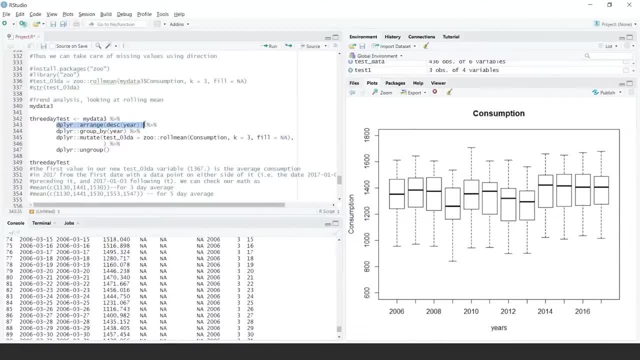 and you can see the result of this. so I am going to arrange this data in descending order of year, so obviously my last one, 2017 or 2018, will be on the top. you want to group the data by year, so it depends on how many years we have. 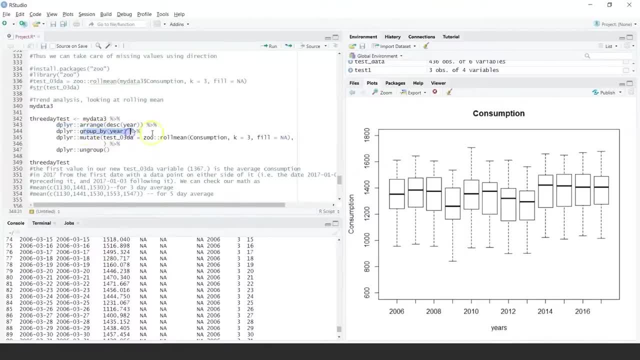 we will see. so you can group the data by year. now this data is then used to basically mutate. so mutate function is going to allow me to use this rolling mean, so I will call it as says 03 day. so I am going to calculate a rolling mean every 3 days. 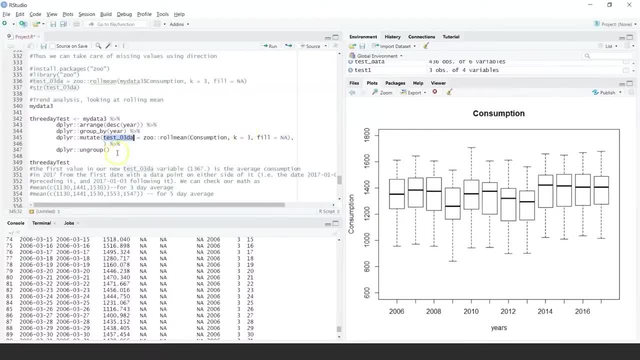 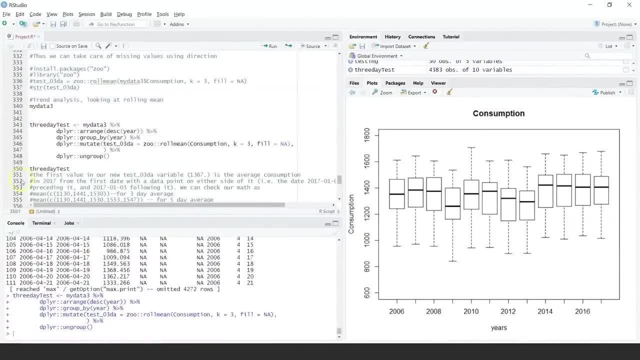 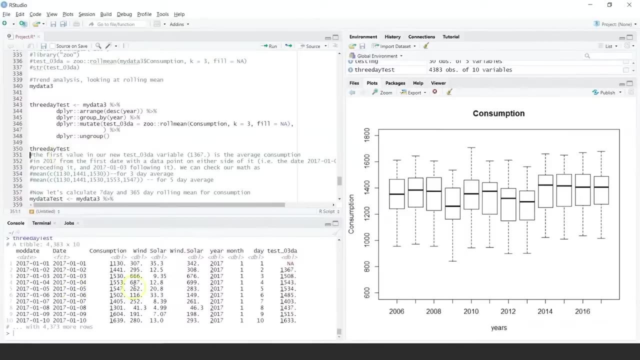 for my consumption column and basically, let's ungroup this so let's see how this works. sorry, let's look at this and here, when I am doing a 3 day test, let's look at the result of this and then I will explain this. so if you see here, 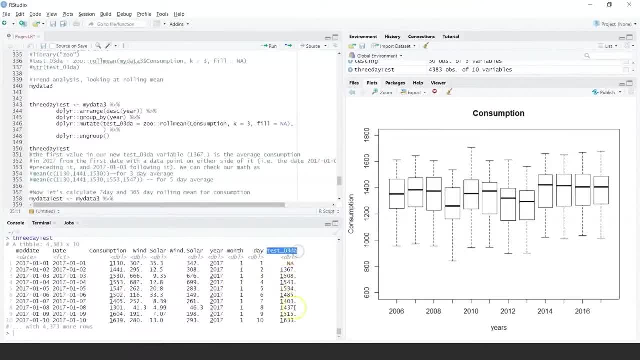 we have the test 3 day column. now this has the rolling average. now, what does that mean? so, first value here, what we see is 1367 is the average consumption in 2017, from the first date, with the data point on either side of it, that 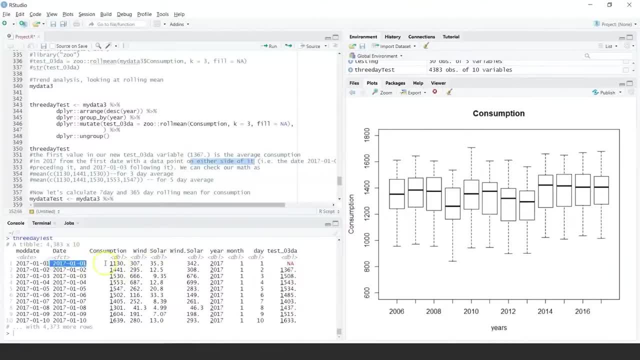 is. you can look at this date, so 1130. then you look at, you are looking at the value 1367 here, so you look at 1130, 1441, 1530, if I take a mean of these. so, for example, if I would just do this part, 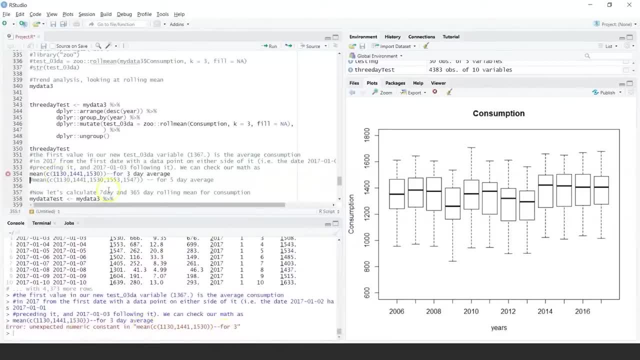 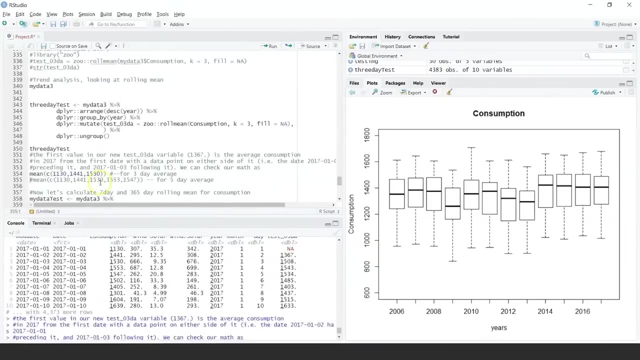 and that is giving me mean okay, because I have a comment, so let's basically add anything as comment and then let's do this. so it says me 1367. that's what we are seeing here, right? so you are getting a rolling average every 3 days. 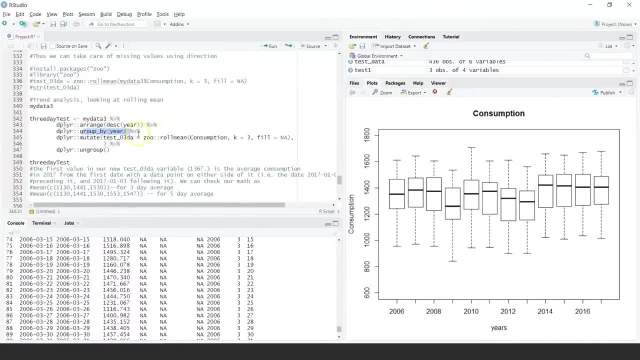 so you can group the data by year. now this data is then used to basically mutate. so mutate function is going to allow me to use this rolling mean, so I will call it as says 03 day. so I am going to calculate a rolling mean every 3 days. 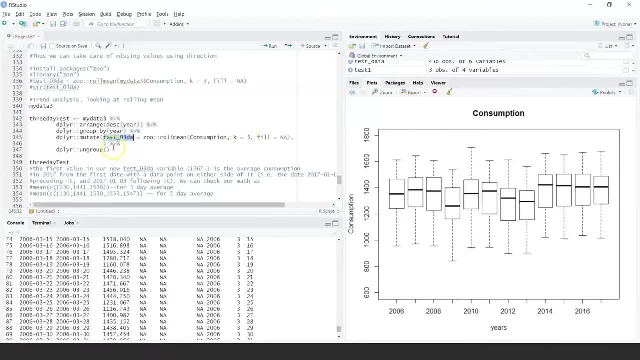 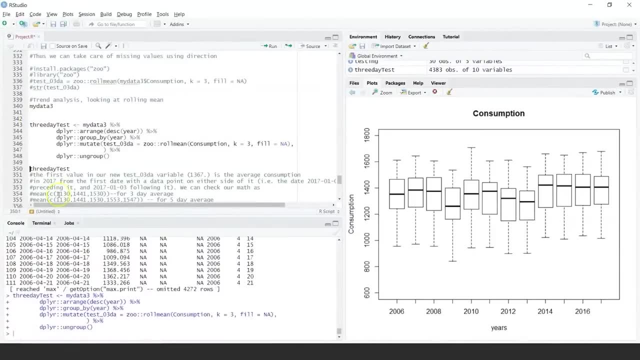 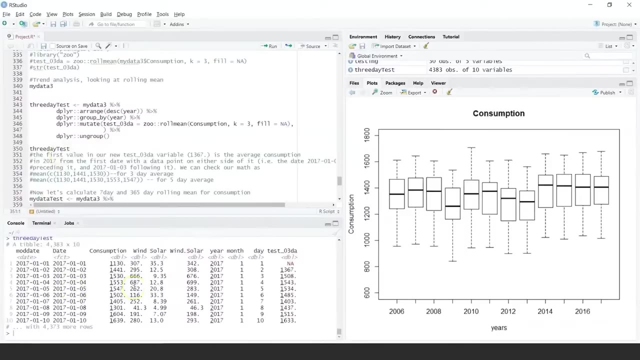 for my consumption column and basically, let's ungroup this so let's see how this works, sorry, yeah, let's look at this. and here, when I am doing a 3 day test, let's look at the result of this and then I will explain this. so if you see here, 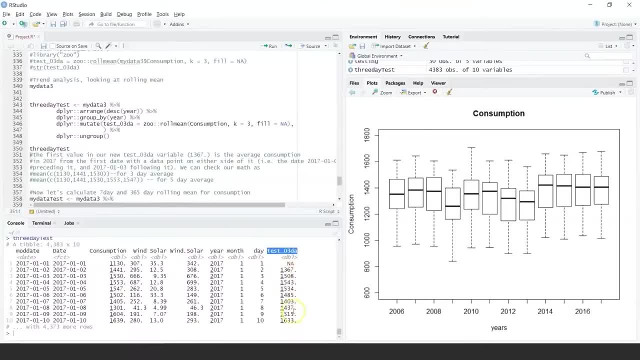 we have the test 3 day column. now this has the rolling average. now, what does that mean? so, first value here, what we see is 1367 is the average consumption in 2017, from the first date, with the data point on either side of it, that is. 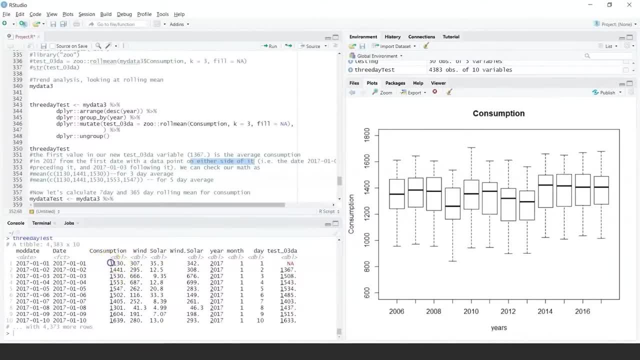 you can look at this date, so 1130. then you look at, you are looking at the value 1367 here, so you look at 1130, 1441, 1530, if I take a mean of these. so, for example, if I would just do this part, 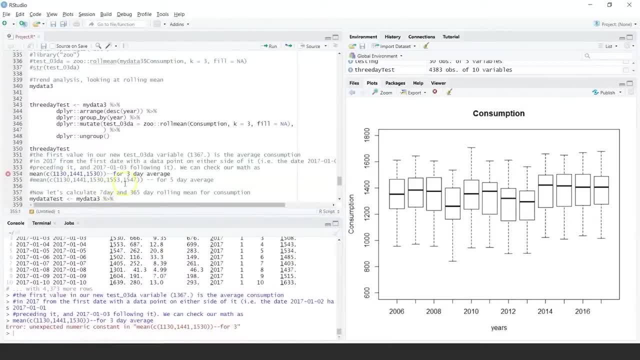 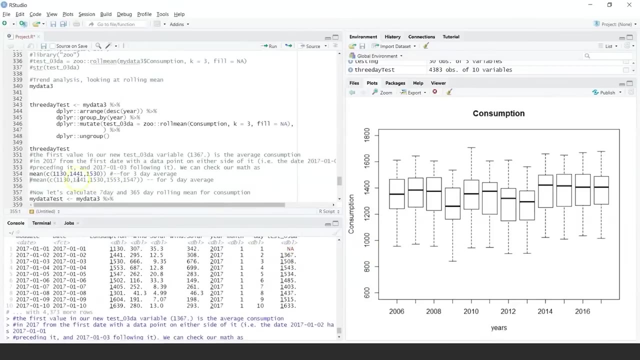 and that is giving me mean ok, because I have a comment, so let's basically add anything as comment and then let's do this. so it says me 1367. that's what we are seeing here, right? so you are getting a rolling average every 3 days. similarly, 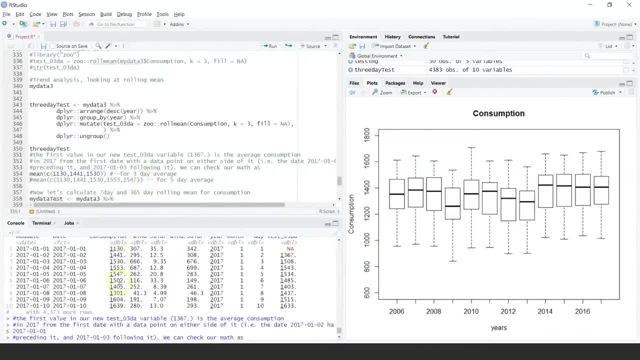 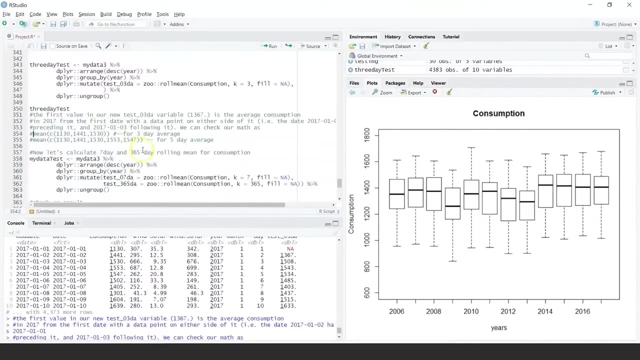 similarly, if you want every 5 days, it takes the 5 values and it gets the mid value right, so you can always find out the mean, rolling mean, for a particular frequency. now let's do that for 7 days. that is weekly data and yearly data, that is. 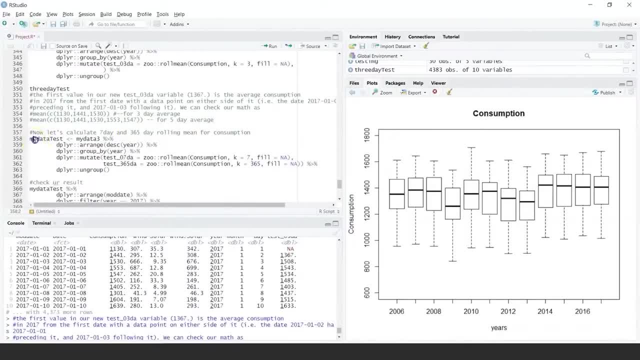 365 days. so how do I do it same logic, my data test. now I am using my data 3. I am arranging it in a descending order. I am grouping by year. so when you do a group by year. so earlier when we did a grouping by 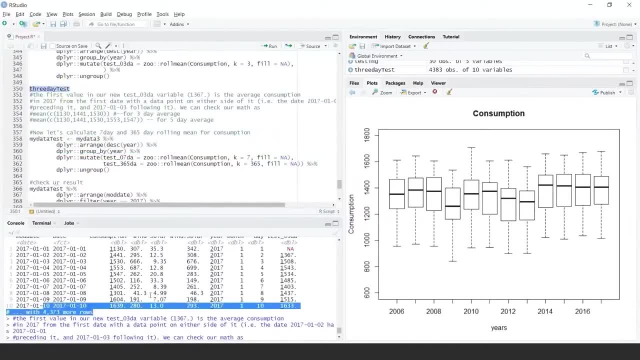 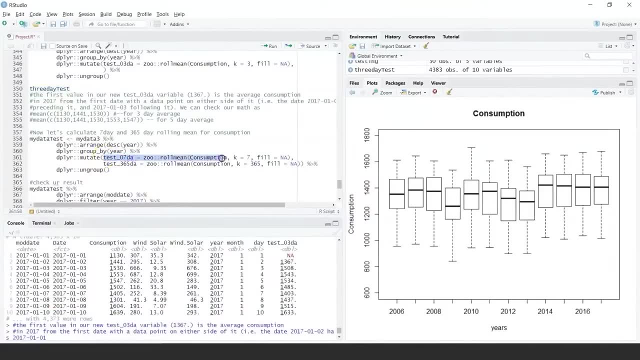 and when we looked at the data it was telling me how many rows we had right. so let's do a grouping by year and let's say test 07. so that's rolling average every 7 days. and I am also saying: take care of the NA values. 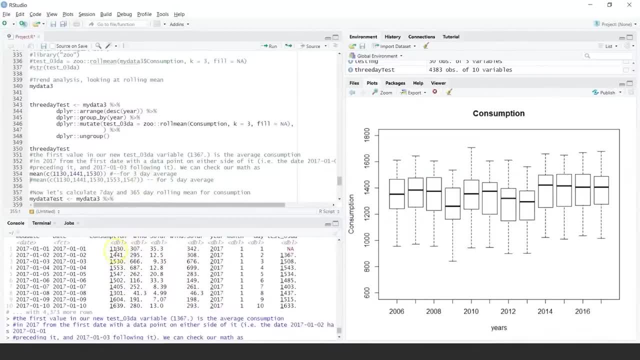 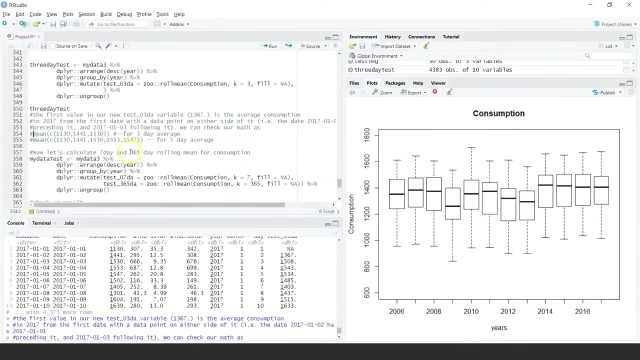 if you want, every 5 days, it takes the 5 values and it gets the mid value right, so you can always find out the mean, rolling mean, for a particular frequency. now let's do that for 7 days. that is weekly data and yearly data, that is. 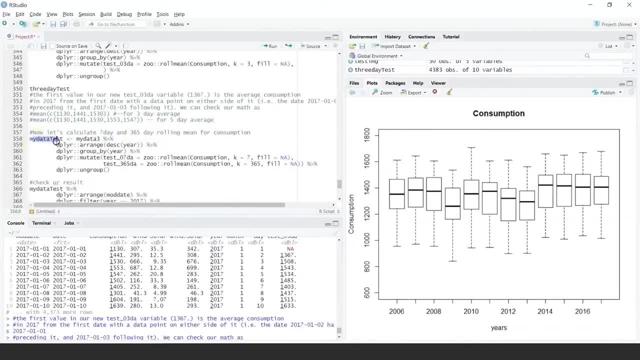 365 days. so how do I do it same logic, my data test. now I am using my data 3. I am arranging it in a descending order. I am grouping by year. so when you do a group by year, so earlier when we did a grouping by and when we 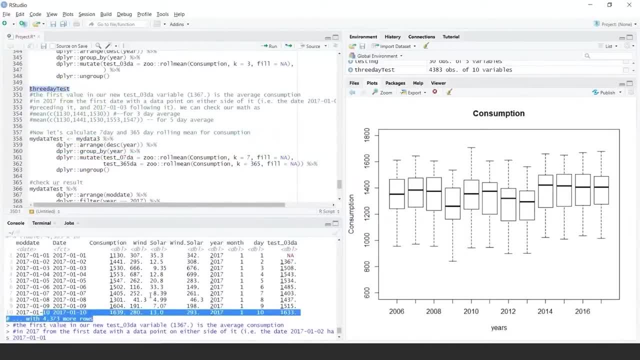 looked at the data, it was telling me how many rows we had. so let's do a grouping by year and let's say test 07. so that's a rolling average every 7 days. and I am also saying: take care of the NA values. similarly, I am getting rolling average every. 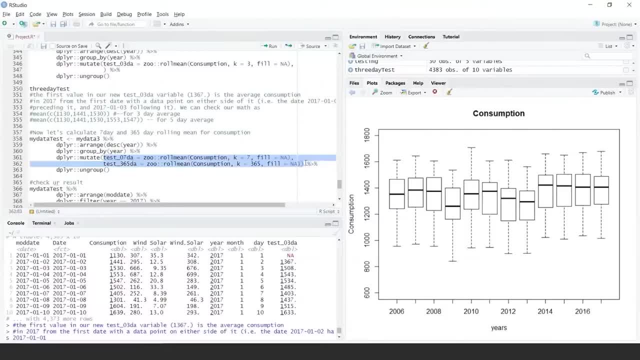 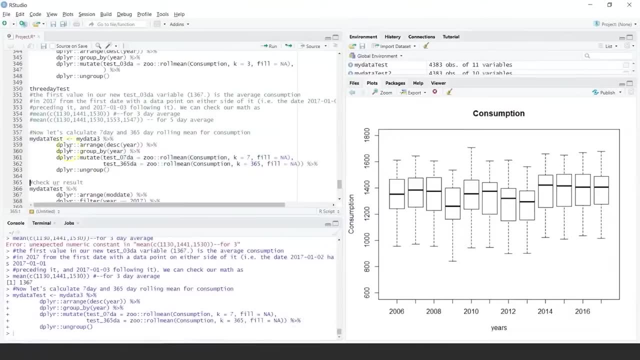 similarly, I am getting rolling average: 365 days. might be you can do quarterly, might be you can do half yearly, and let's do this. so let's create this my data test and let's look at the result of this. so I will use my data test. 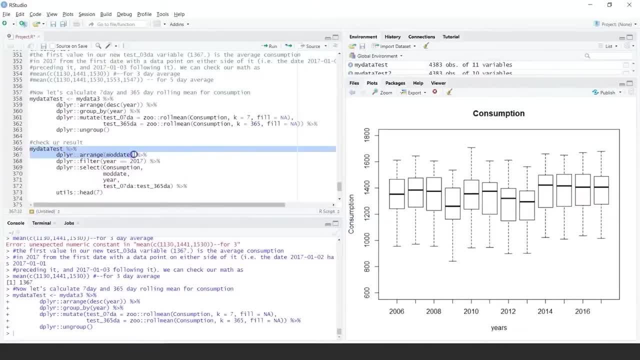 I will say: arrange based on modified date. now we know there is a column called modified date. I want to just look at 2017 data, so I am doing a filter, right, and then I will choose what are the columns I am interested in. so I will look at the. 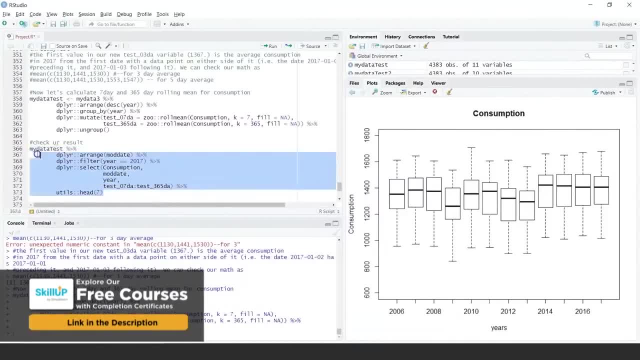 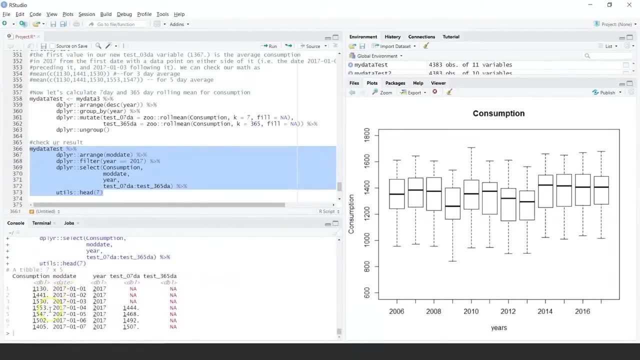 7 and 365 day and let's look at, say, first 7 records, so let's do this, and that basically gives me the consumption value modified date, year and my rolling 7 day average, or the 7 day mean, which is for first 7 days and then 365. 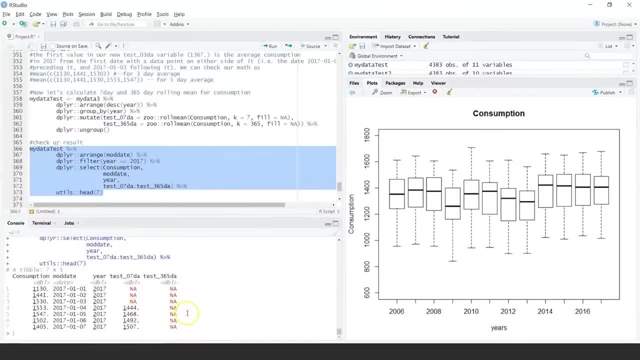 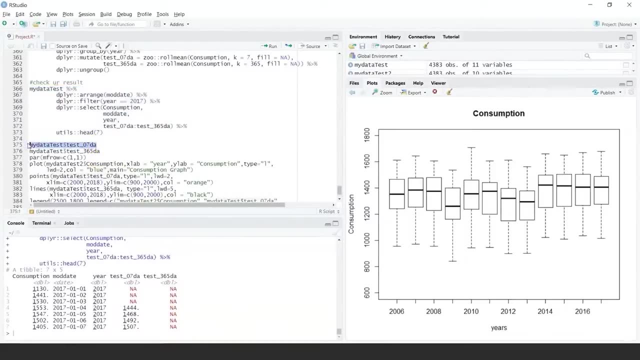 you will not see the data here, but if I do a view on this, I can basically see the values, so you can always select a particular column to see the values. these are the values for every 7 day rolling average. this is for 365 days, every 365. 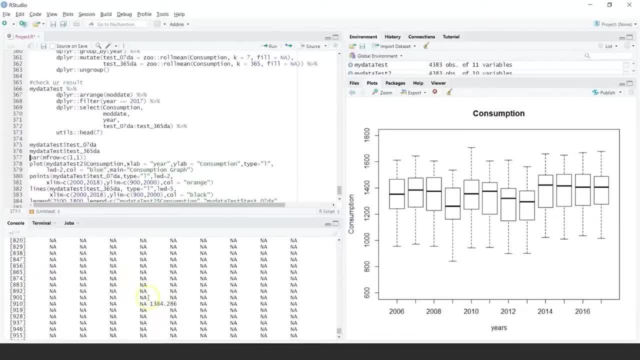 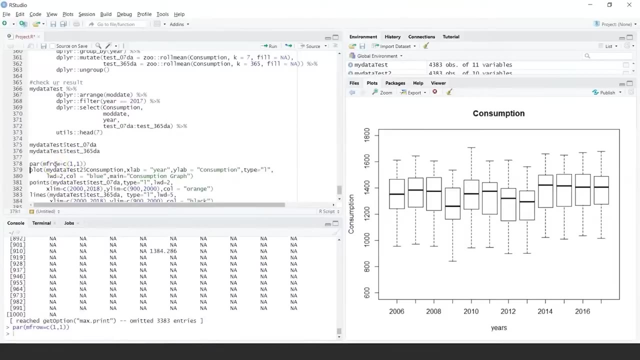 days. so you see all the values are missing. but every 365 entry you will have basically some data. now let's do a plotting of this and basically visualize this data which we are seeing rolling average. so let me first do a plotting, one plot per graph and 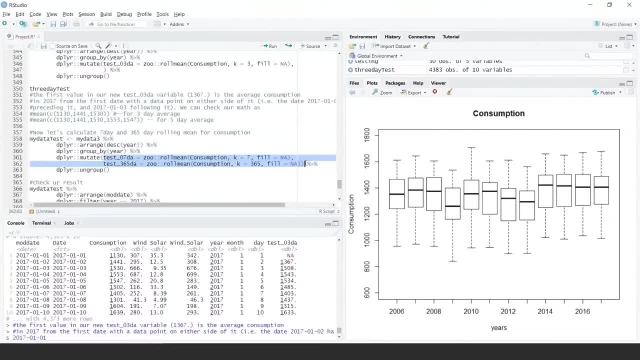 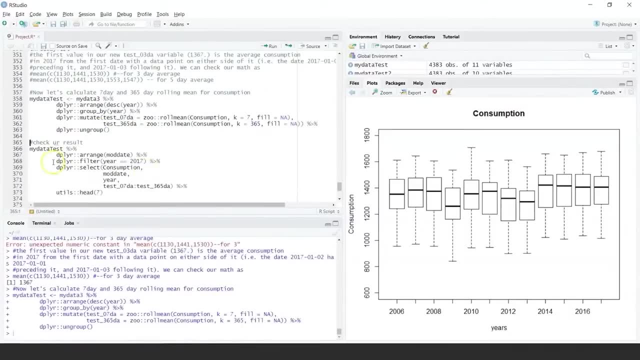 365 days might be. you can do quarter yearly. might be you can do half yearly and let's do this. so let's create this my data test and let's look at the result of this. so I will use my data test. I will say: arrange based. 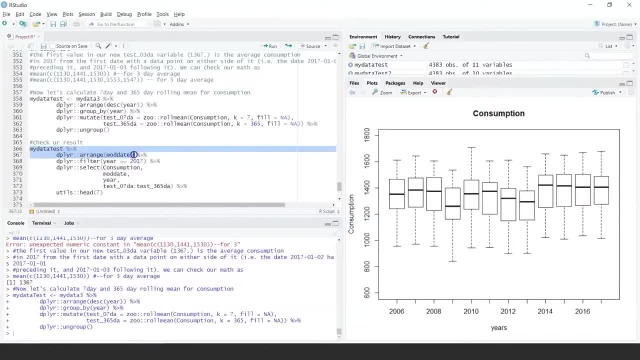 on modified date. now we know there is a column called modified date. I want to just look at 2017 data, so I am doing a filter right, and then I will choose what are the columns I am interested in. so I will look at the 7. 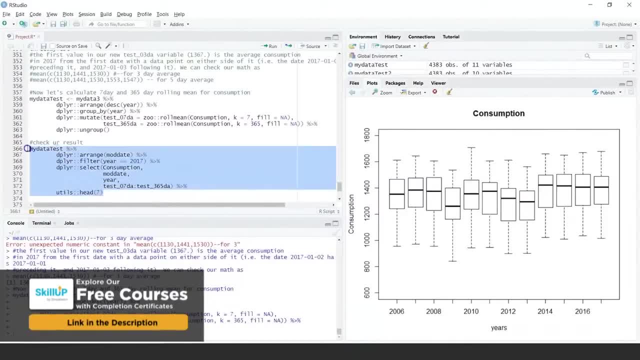 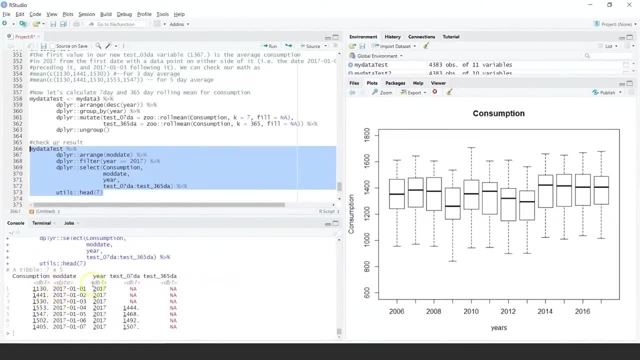 and 365 day and let's look at, say, first 7 records, so let's do this and that basically gives me the consumption value modified date, year and my rolling 7 day average or 7 day mean, which is for first 7 days and then 365. you 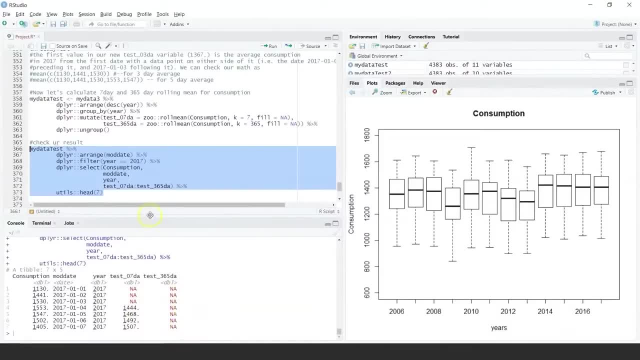 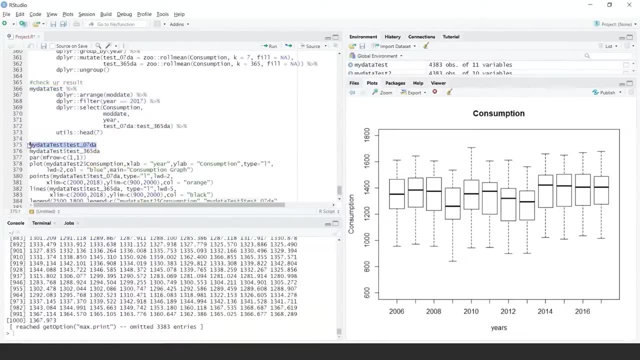 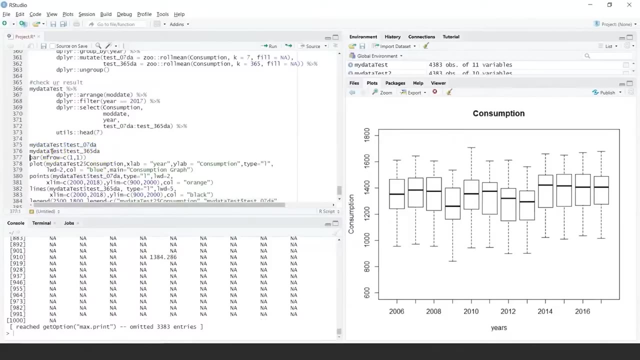 will not see the data here, but if I do a view on this, I can basically see the values, so you can always select a particular column to see the values. these are the values for every 7 day rolling average. this is for 365 days, every 365. 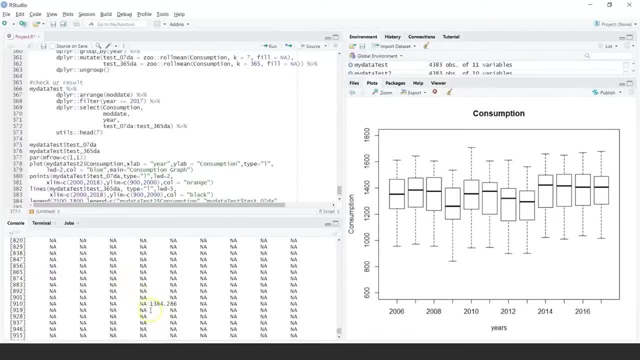 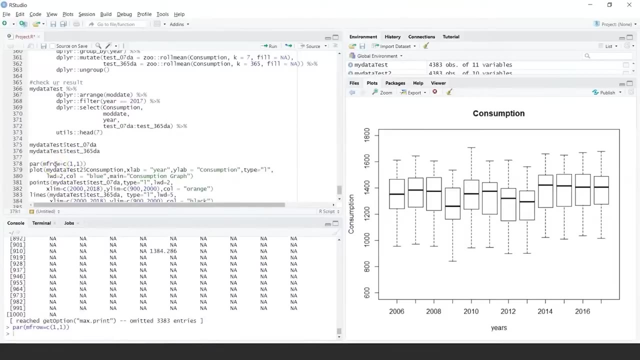 days. so you see all the values are missing. but every 365 entry you will have basically some data. now let's do a plotting of this and basically visualize this data which we are seeing rolling average. so let me first do a plotting- one plot per graph- and let's do 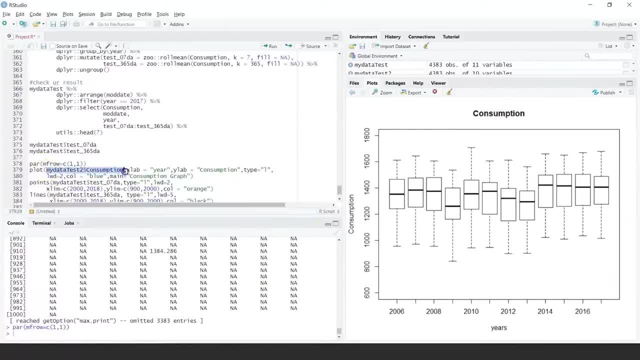 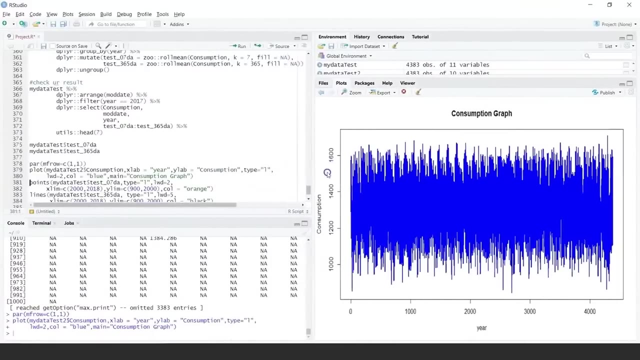 let's do a plotting. I will take consumption data- x axis, y axis, color- and give a title to this. so let's create this and that's my consumption data, which is spread over a period of time, and that's fair enough. but now let's add some. 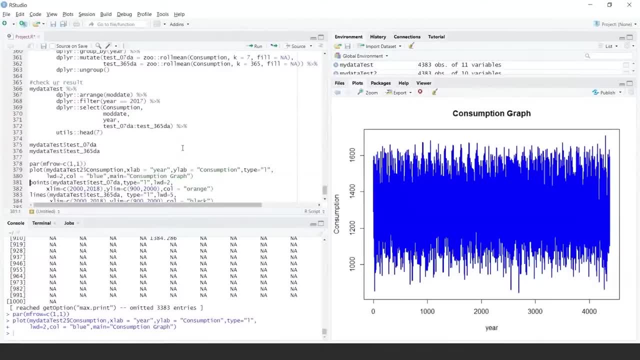 more plot to this. so I will add the 7 day rolling average to this. so for second plot to be added in the same one in R you can use points. so I will say points. I will choose 7. data column type is line width x, limit y. 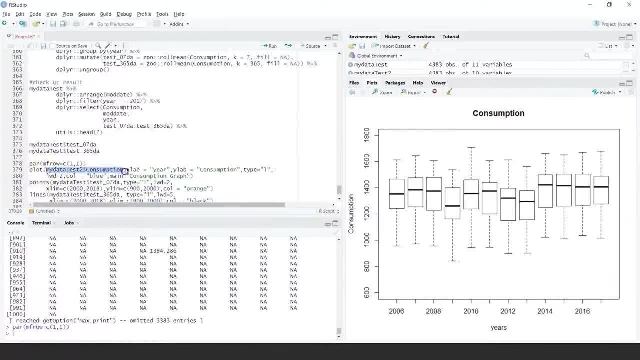 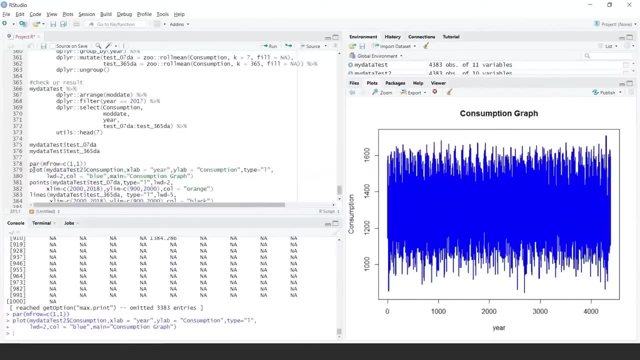 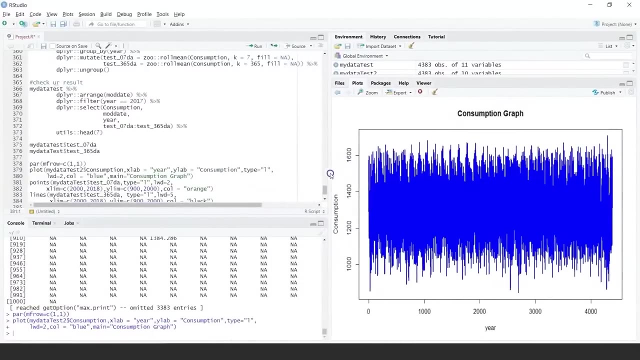 a plotting. I will take consumption data x-axis, y-axis, color and give a title to this. so let's create this and that's my consumption data, which is spread over a period of time, and that's fair enough. but now let's add some more plot to this. so I will add the. 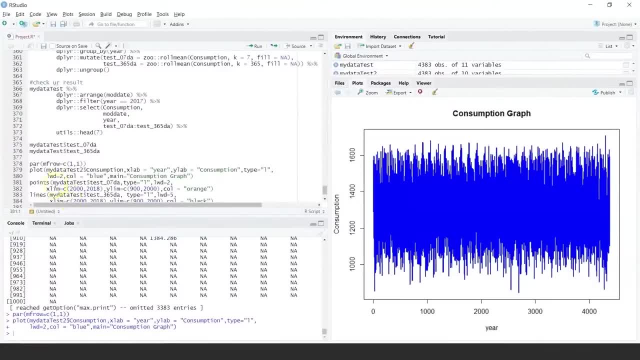 7 day rolling average to this. so for second plot to be added in the same one in R you can use points. so I will say points. I will choose 7. data column type is line width, x, limit, y, limit and color. so let's do this. 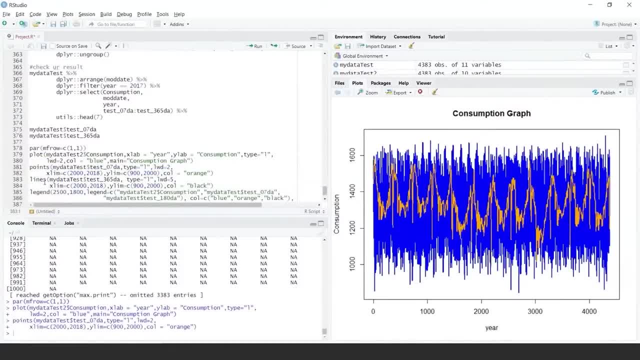 limit and color. so let's do this, and that's my pattern: 7 day rolling average, which basically gives me some kind of trend. similarly, I can add one more here, and this time I will choose the 365 and look at the pattern lines. so now you see some dots. 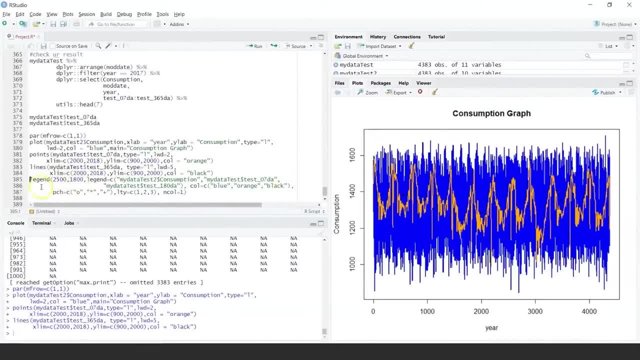 here. well, you could do it in a different way. so I can just add legend to this and I can say: legend will be aware in x axis and y axis. so I am saying it will be 2500 and y is 1800. so my legend will come in some in. 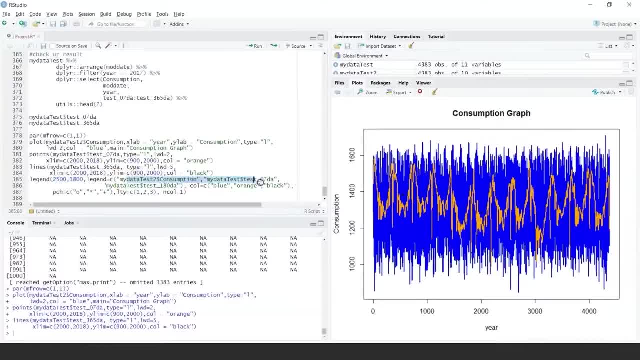 here I am saying my legend will have consumption test and this one I can give some names, I can give what is the color, I can say what kind of legend it explains what is for each color and then basically a vector. so let's add a legend to this and I have added a legend. 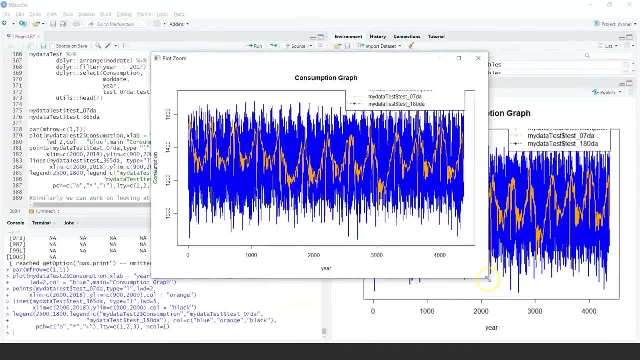 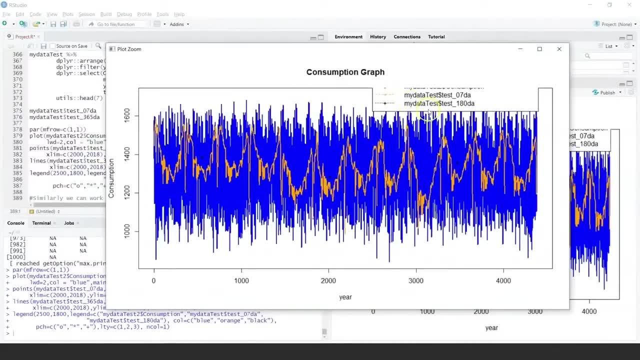 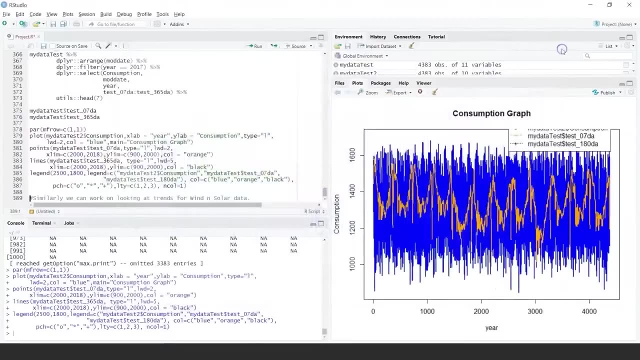 now you can do a zoom and look at the data, and here I see that my x axis is fine but y axis is going a little about of my plotting area, so I can actually change that. so here I have 1800. how about making it 1600? 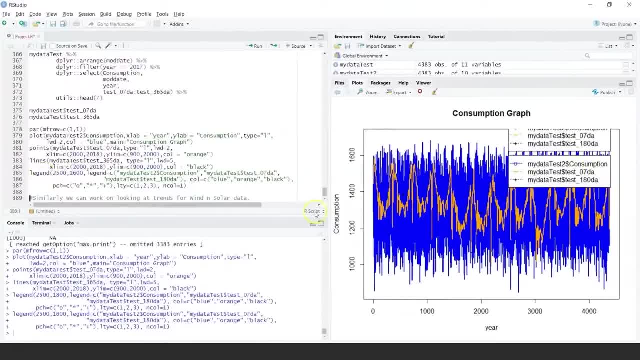 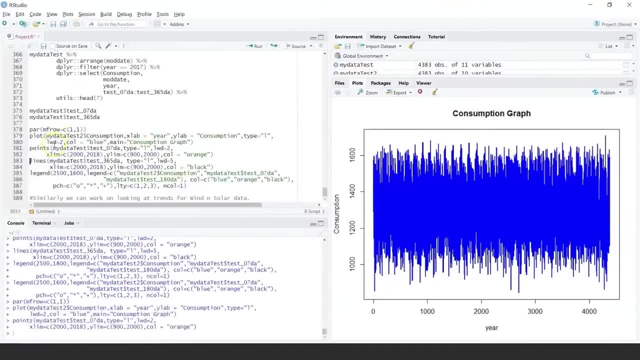 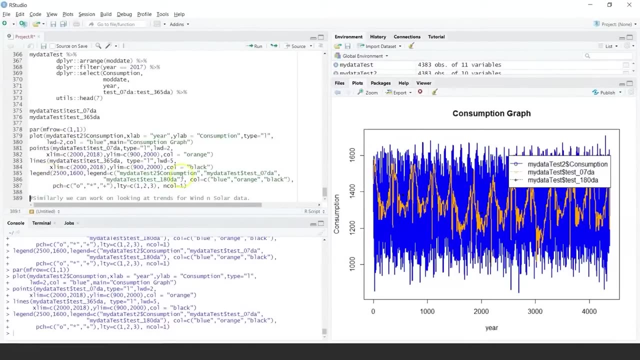 and let's look at this one. so we can basically go for this one and start again here, plot and points and line, and then add a legend. right, and you can basically place your legend anywhere in the plot. so this basically is giving me the trend, what I am. 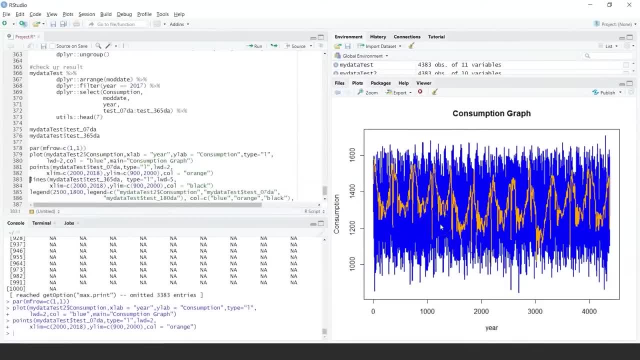 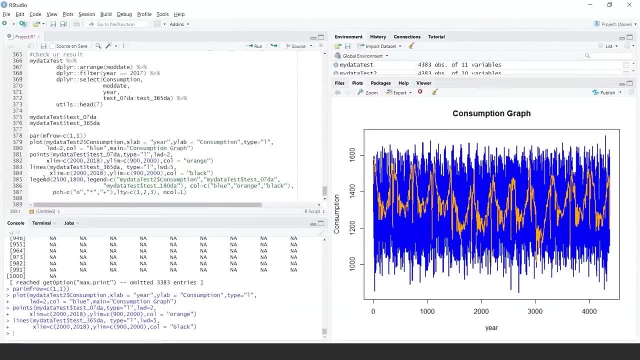 and that's my pattern: 7 day rolling average, which basically gives me some kind of trend. similarly, I can add one more here, and this time I will choose the 365 day and look at the pattern lines. so now you see some dots here. well, you could do it in a different way. 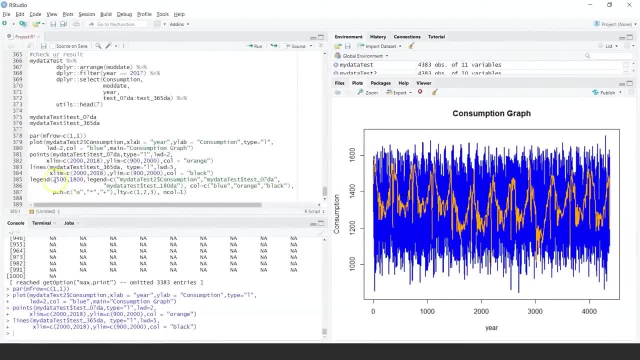 so I can just add legend to this and I can say legend will be aware in x-axis and y-axis. so I am saying it will be 2500 and y is 1800. so my legend will come in somewhere here I am saying my legend will. 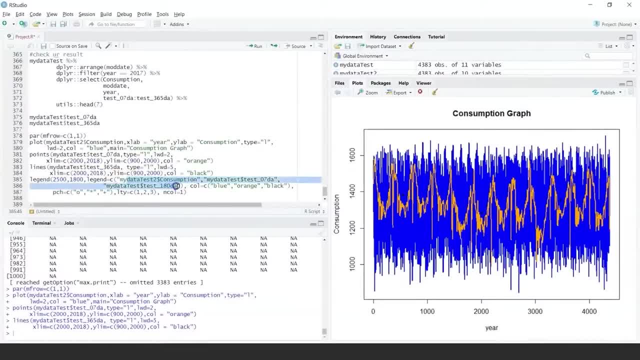 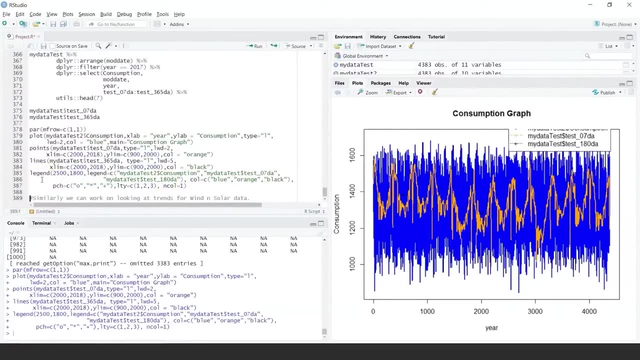 have consumption test and this one. I can give some names, I can give what is the color, I can say what kind of legend it explains what is for each color and then basically a vector. so let's add a legend to this, and I have added a legend. 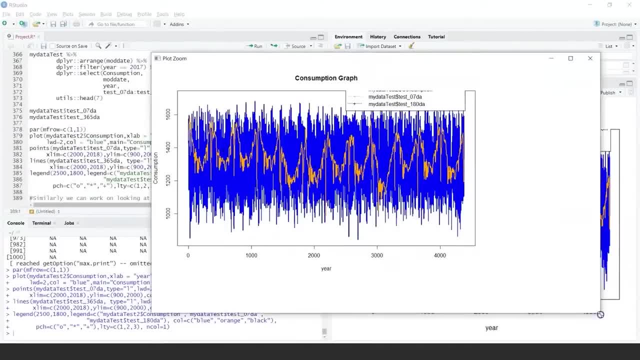 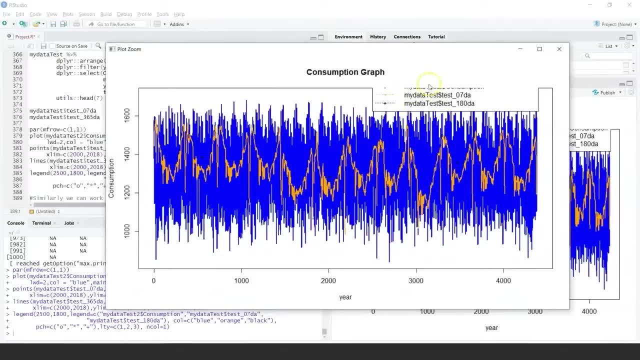 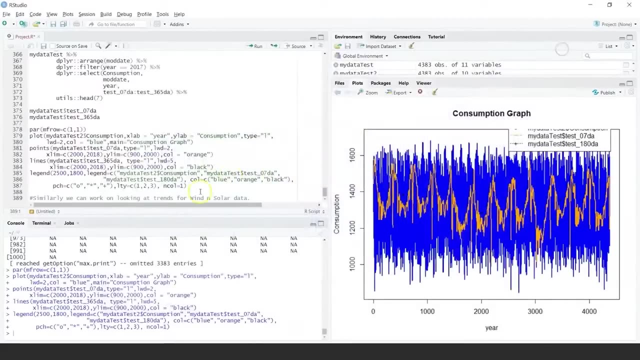 now you can do a zoom and look at the data, and here I see that my x-axis is fine but y-axis is going a little about of my plotting area, so I can actually change that. so here I have 1800. how about making it 1600? 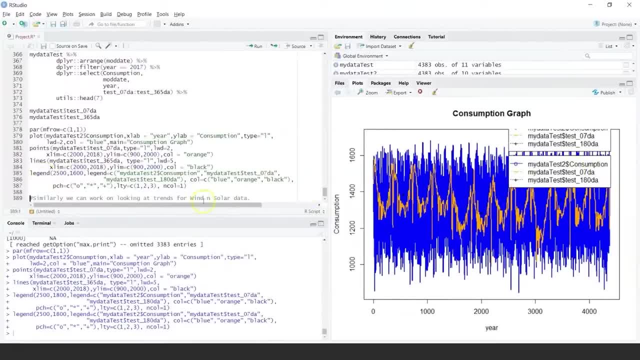 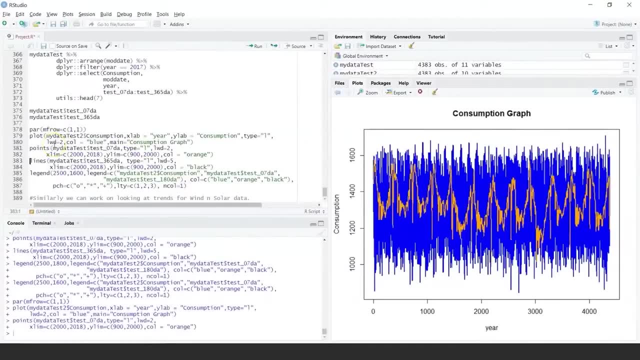 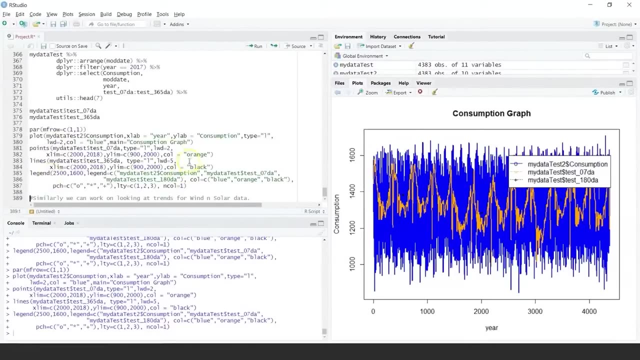 and let's look at this one. so we can basically go for this one and start again here, plot and points and line, and then add a legend. right, and you can basically place your legend anywhere in the plot. so this basically is giving me the trend, what I am looking. 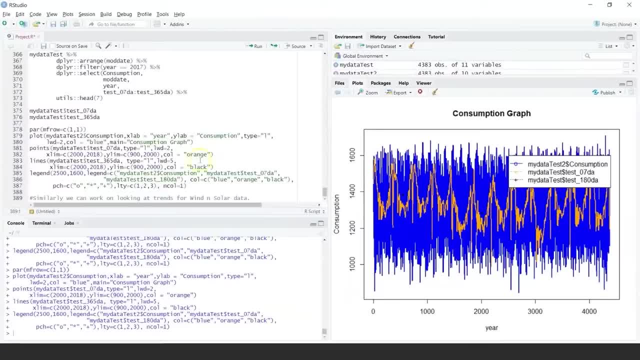 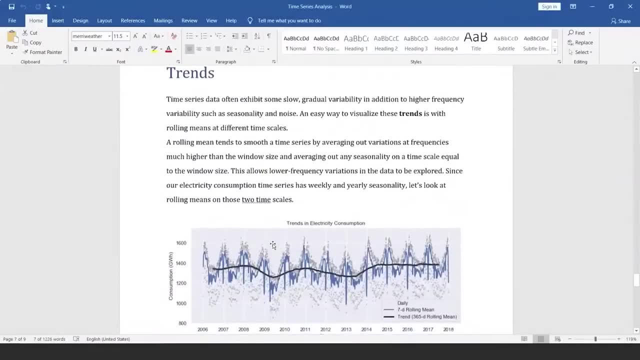 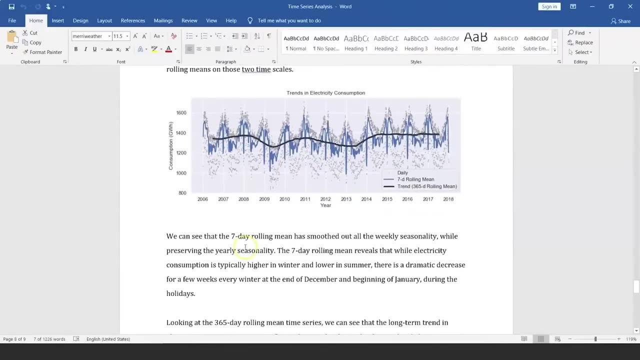 at my rolling average. so similarly you can look at the trend for wind and solar data. so what we are seeing here is when you look at trend. this is one more way of looking at it. you can always create plots in different ways. so 7 day rolling mean has: 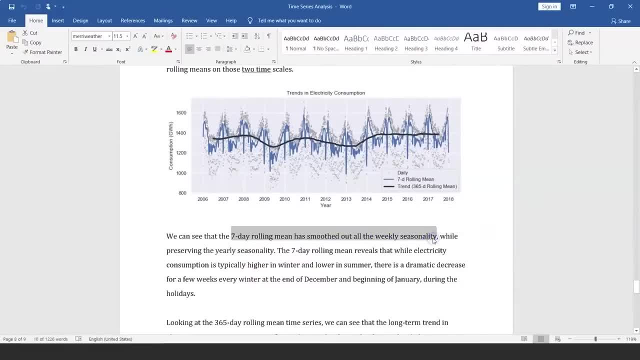 smoothed out all week seasonality which we were seeing here in my graph where you look at every 7 day, preserving the yearly seasonality. so 7 day will tell that electricity consumption is typically higher in winter and lower in summer, so better is you break it down yearly. 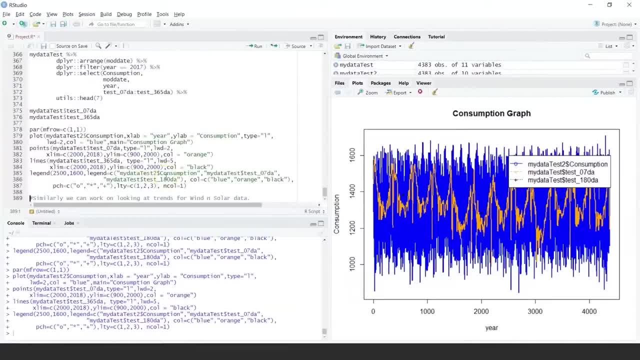 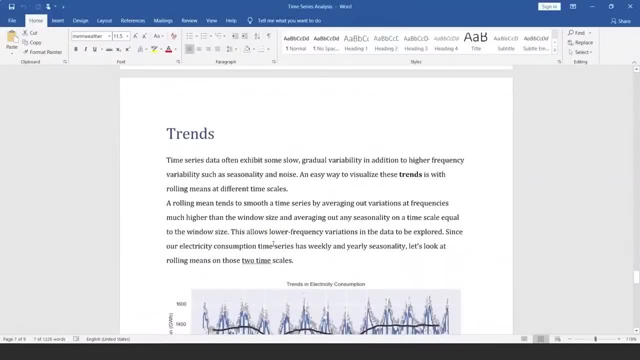 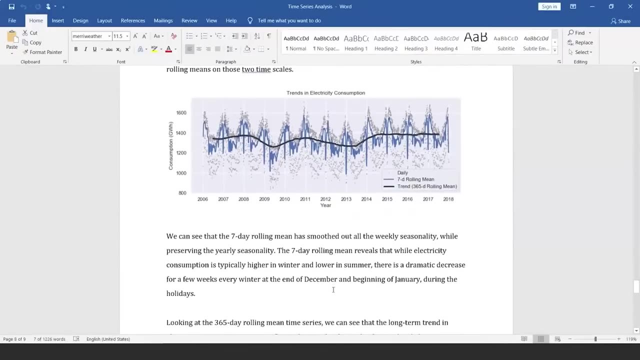 looking at my rolling average. so similarly, you can look at the trend for wind and solar data. so what we are seeing here is when you look at trend. this is one more way of looking at it. you can always create plots in different ways. so 7 day rolling mean. 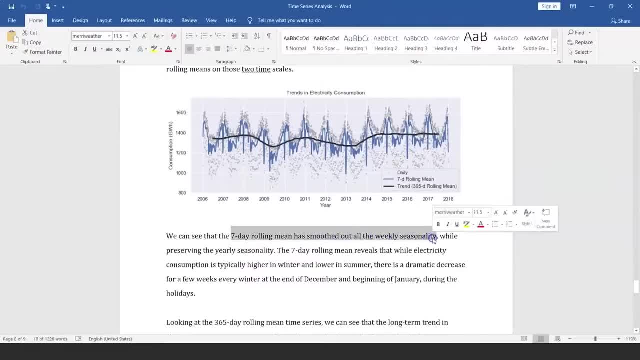 has smoothed out all week seasonality which we were seeing here in my graph where you look at every 7 day, preserving the yearly seasonality. so 7 day will tell that electricity consumption is typically higher in winter and lower in summer. so better is you break it down. 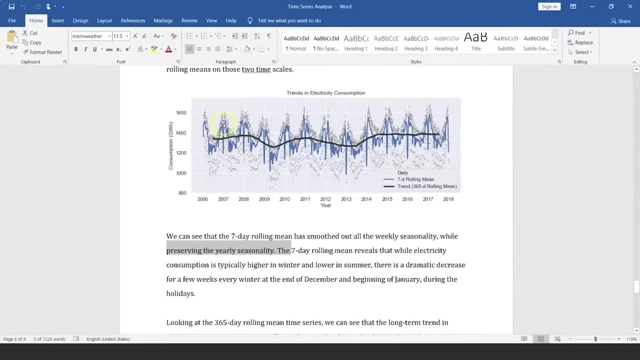 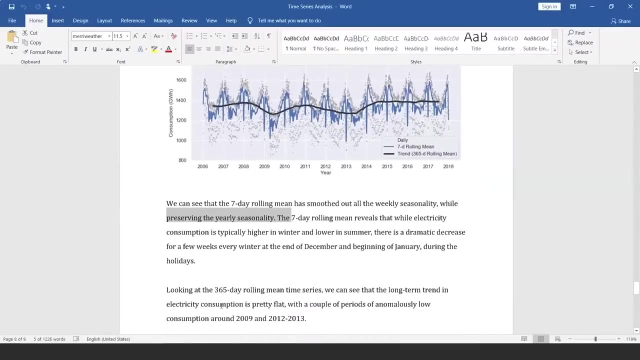 yearly. so here, if you look at every year, you can see when is winter, when is summer, what is the seasonality, what your trend, what you are seeing here, and if there is a decrease or increase for few weeks every winter. so, similarly, if you look at 365 now, as you said, as 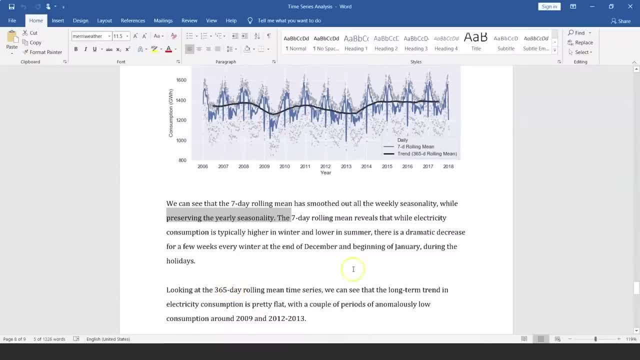 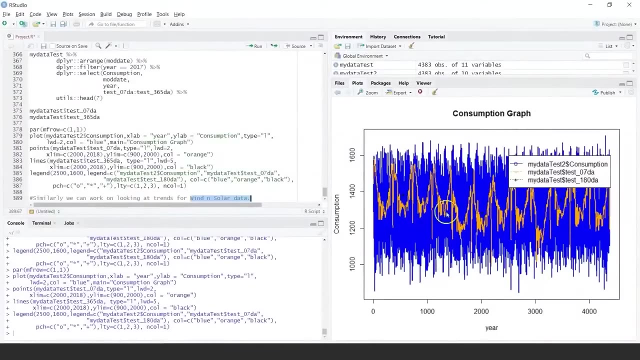 I said, rolling average basically reduces the variation. so if I look at 365 rolling mean we can see long term trend in electricity consumption is pretty flat. now that's what we are seeing. it's kind of pretty flat. there is not much variation over years, if you really 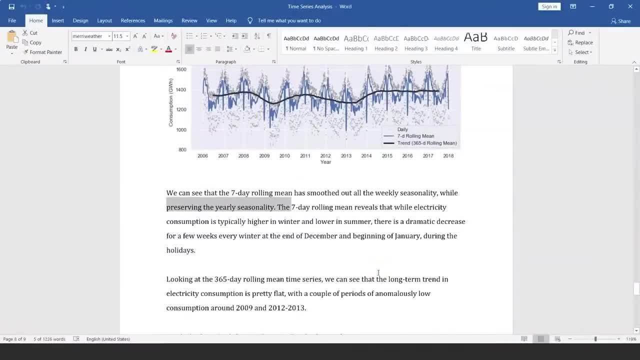 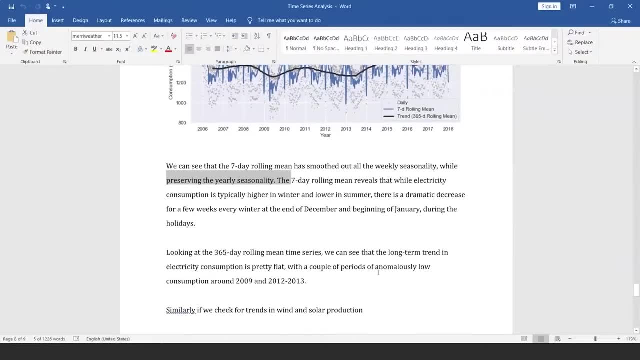 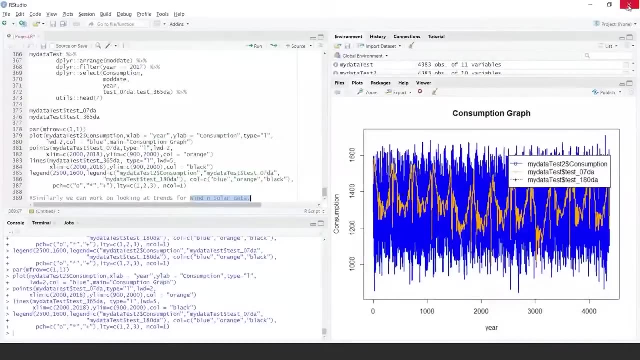 join these dots so we can basically see some highs and lows, and that gives me a trend. now this is how you can do a trend detection, and similarly we can do plotting for wind and solar. so this is a small project which I demonstrated using R. now all. 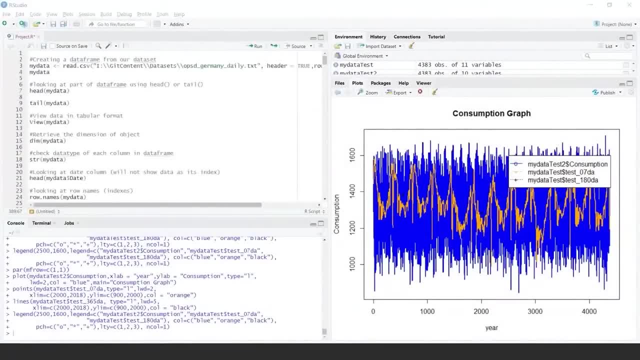 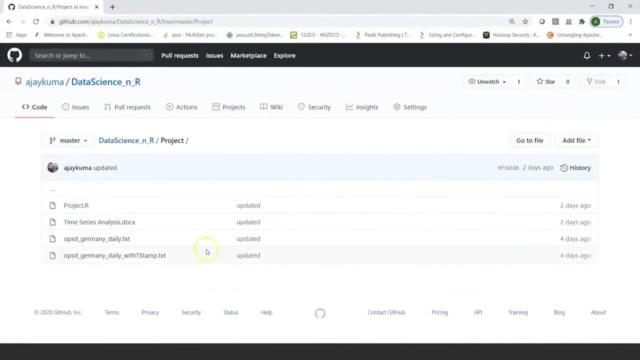 this code, which you have here in the form of a project dot R file you can find here in my github page. this is the document which explains some things. feel free to download this and you can add details to it. this is the sample data set, which you can also find. 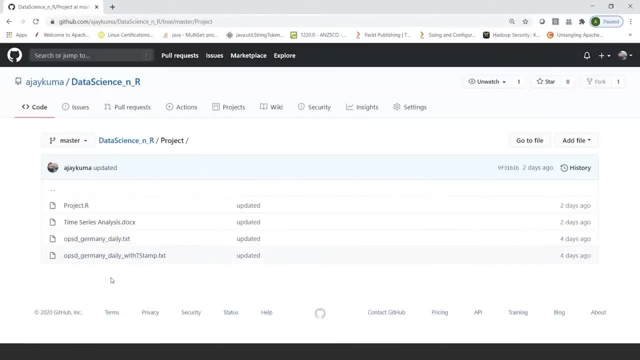 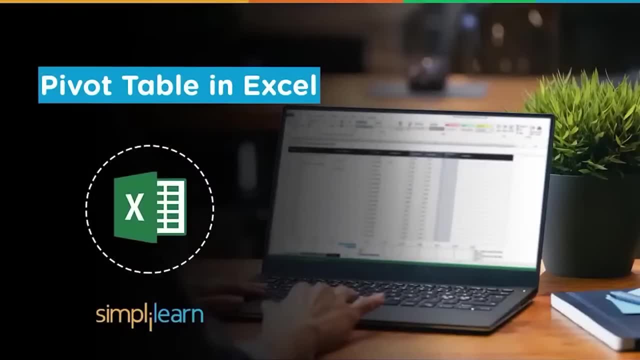 in my repository in the data sets folder. so continue learning and continue practicing. R Excel is a really powerful tool for data analytics and reporting, and pivot tables are one of the features that excel offers for creating tabular reports to summarize our data, let's begin by understanding what is a 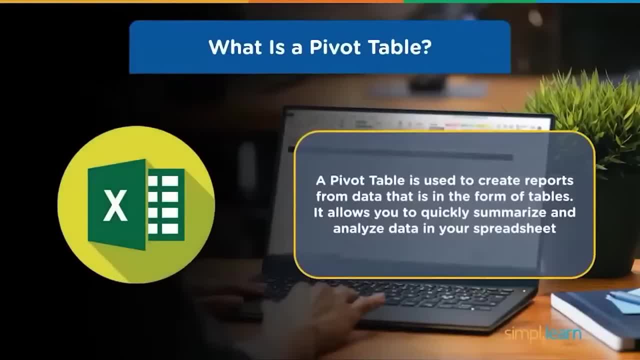 pivot table. a pivot table is a tool that summarizes and reorganizes selected columns and rows of data in a spreadsheet to obtain a desired report. it does not actually change the spreadsheet data. it simply pivots or turns the data to view it in different perspectives. pivot tables are: 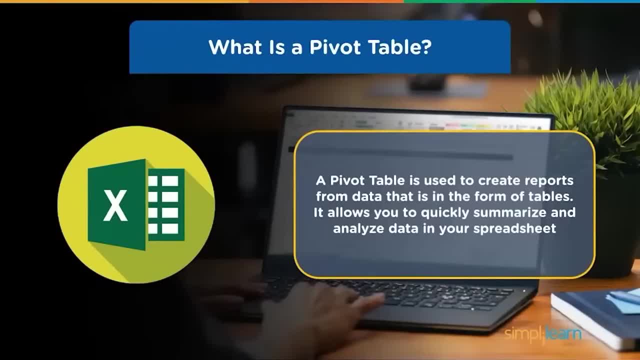 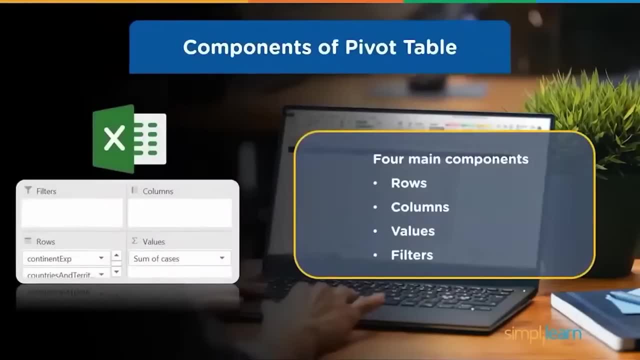 especially useful with large amounts of data that would be time consuming to calculate manually. now let's understand the different components of a pivot table. so there are four main components. first, we have rows. when a field is chosen for the row area, it populates as the first column in the pivot. 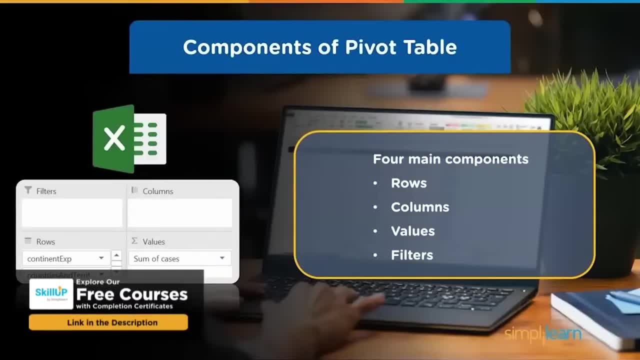 table similar to the columns. all row labels are unique values and duplicates are removed. columns is the second component. when a field is chosen for the column area, only the unique values of the field are listed across the top. then we have values. each value is kept in a pivot table. 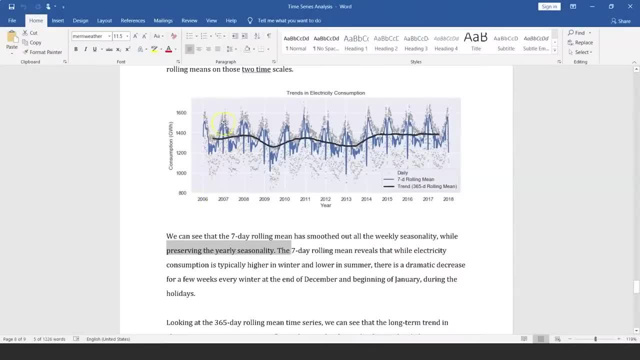 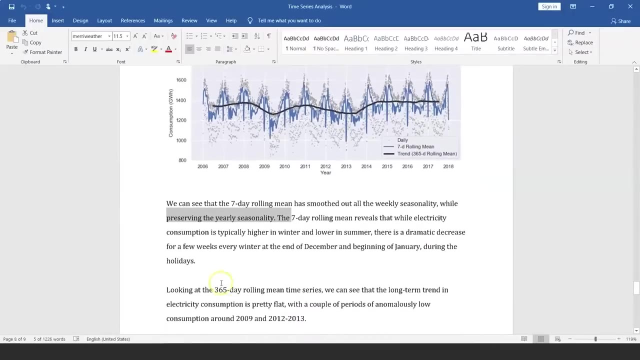 so here, if you look at every year, you can see when is winter, when is summer, what is the seasonality, what your trend, what you are seeing here, and if there is a decrease or increase for few weeks every winter. so, similarly, if you look at 365, 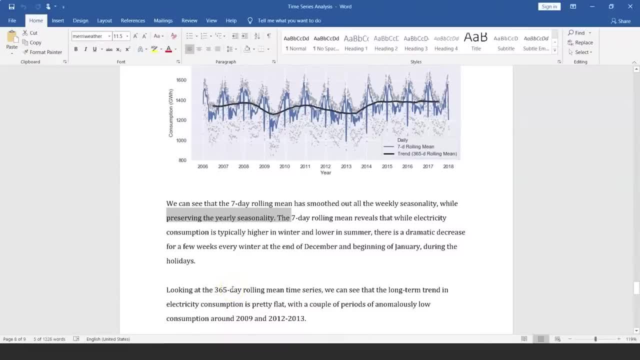 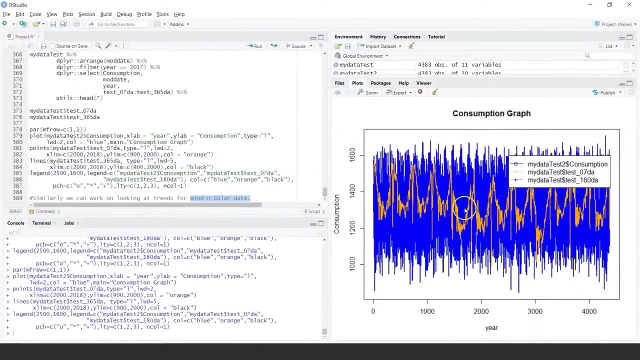 now, as you said, as I said, rolling average basically reduces the variation. so if I look at 365, rolling mean we can see long term trend in electricity consumption is pretty flat. now that's what we are seeing. it's kind of pretty flat, there is not much variation. 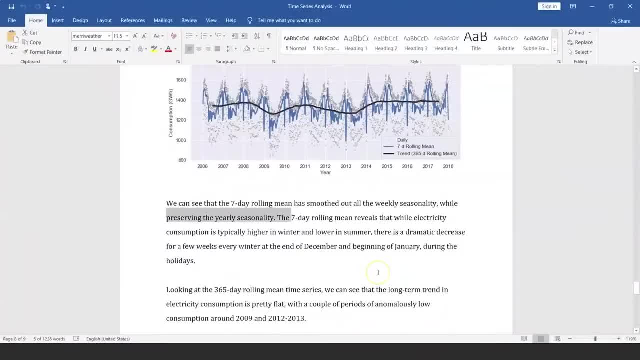 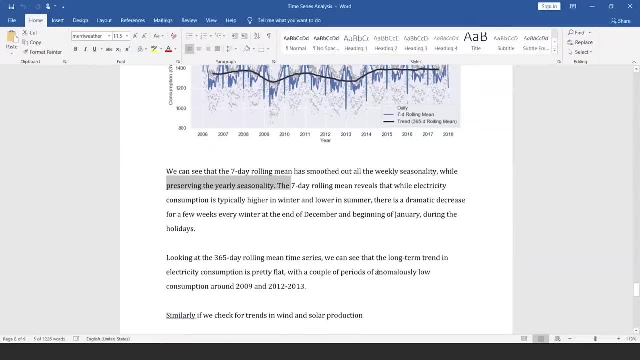 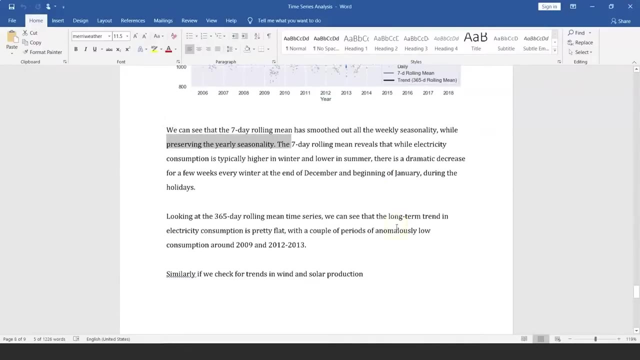 over years, if you really join these dots, so we can basically see some highs and lows, and that gives me a trend. now this is how you can do a trend detection, and similarly we can do plotting for wind and solar. so this is a small project which I demonstrated using 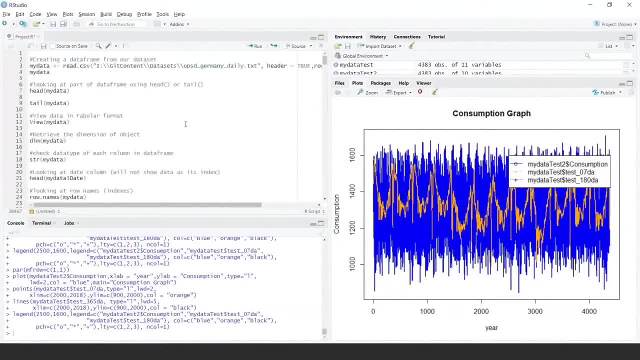 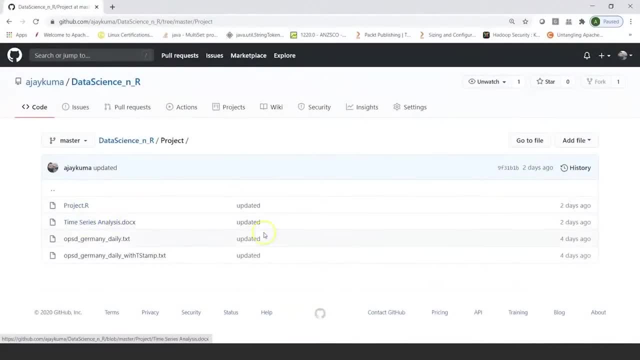 R. now, all this code which you have here in the form of a project dot R file, you can find here in my GitHub page. this is the document which explains some things. feel free to download this and you can add details to it. this is the sample data set, which you can also find in. 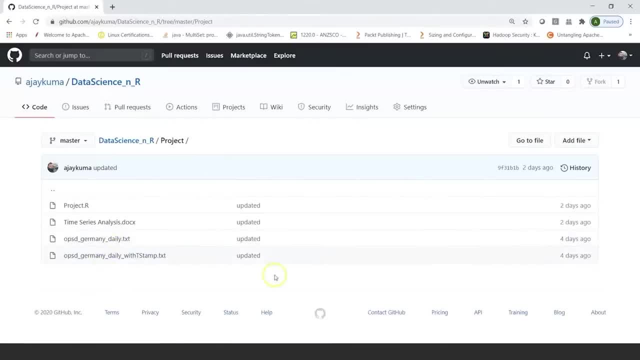 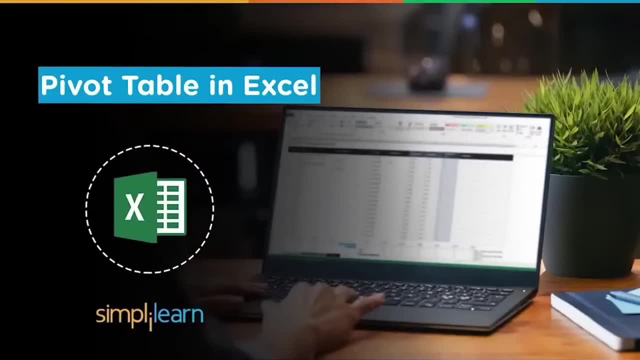 my repository in the data sets folder. so continue learning and continue practicing. R Excel is a really powerful tool for data analytics and reporting, and pivot tables are one of the features that excel offers for creating tabular reports. to summarize our data, let's begin by understanding what is a pivot table. 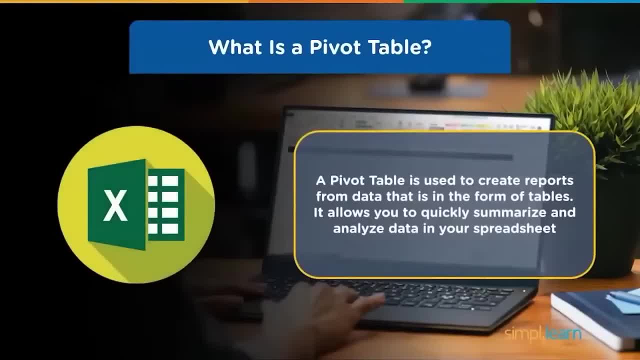 a pivot table is a tool that summarizes and reorganizes selected columns and rows of data in a spreadsheet to obtain a desired report. it does not actually change the spreadsheet data. it simply pivots or turns the data to view it in different perspectives. pivot tables are especially useful. 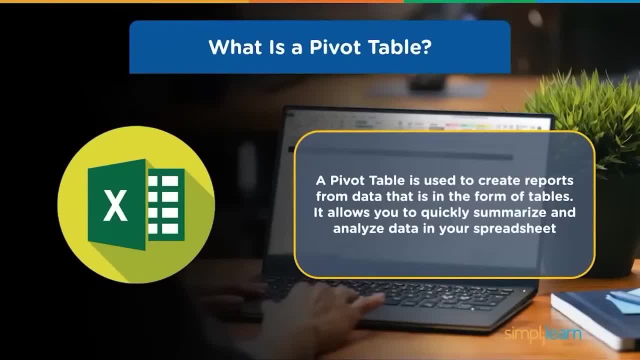 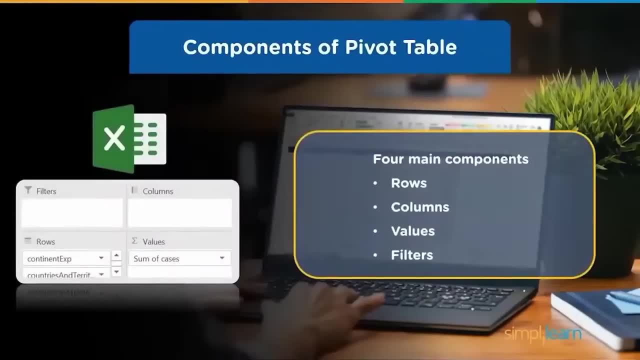 with large amounts of data that would be time consuming to calculate manually. now let's understand the different components of a pivot table. so there are four main components. first, we have rows. when a field is chosen for the row area, it populates as the first column in the pivot table. 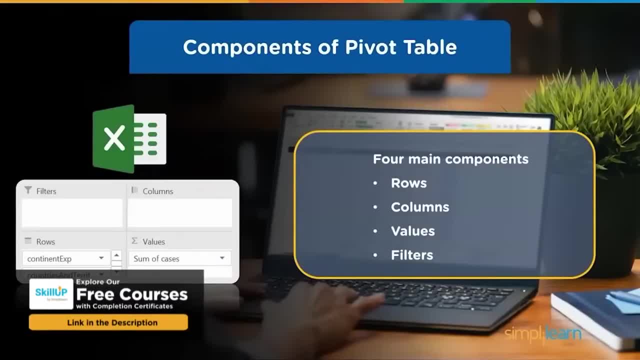 similar to the columns. all row labels are unique values and duplicates are removed. columns is the second component. when a field is chosen for the column area, only the unique values of the field are listed across the top. then we have values. each value is kept in a pivot table cell. 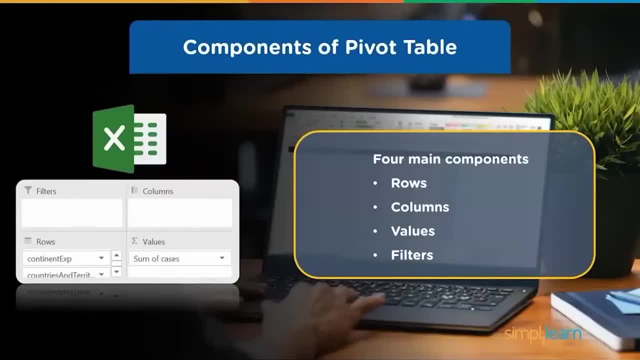 cell and displays the summarized information. the most common values are sum, average, minimum and maximum. finally, we have filters. filters apply a calculation or restriction to the entire table. so let's jump over to microsoft excel and let me show you the data set that we will use in this demo. 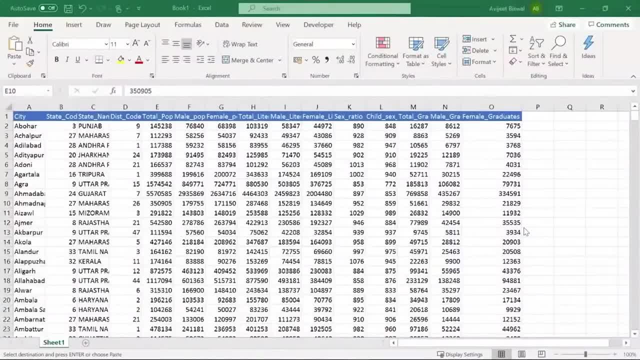 so, with india being ready for its 16th census in 2021- that is, next year- it is a good time for us to analyze india's last census data from 2011 and see where different states and cities across india stood in terms of population literacy and other. 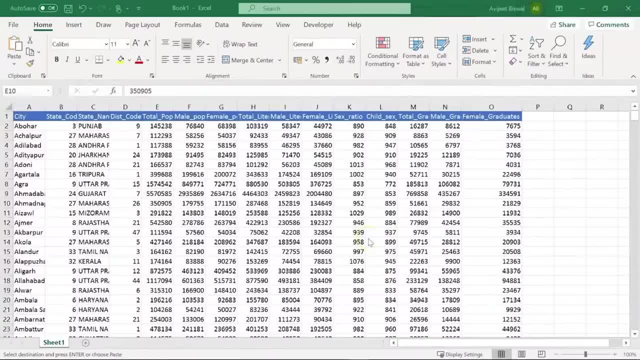 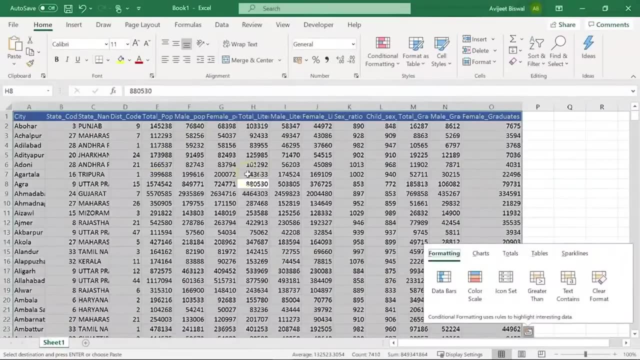 socio-economic factors. we will analyze this data by creating different pivot tables in excel and explore some of its features. so let's begin. first. i'll show you one of the features that excel offers us. so suppose i click on any cell and hit ctrl plus q, you can see our entire table. 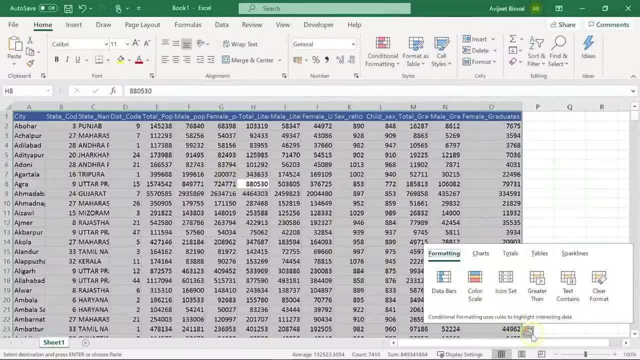 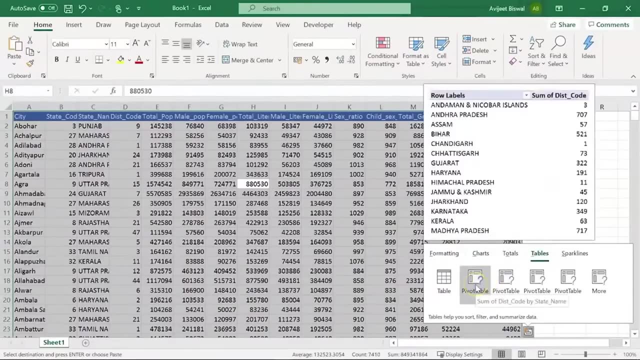 is selected and at the right bottom there's an option of quick analysis. now you can see, by default excel has prompted certain features such as formatting. we have charts, totals and there's one more called tables. now excel by default has created some pivot tables for us. now the first. 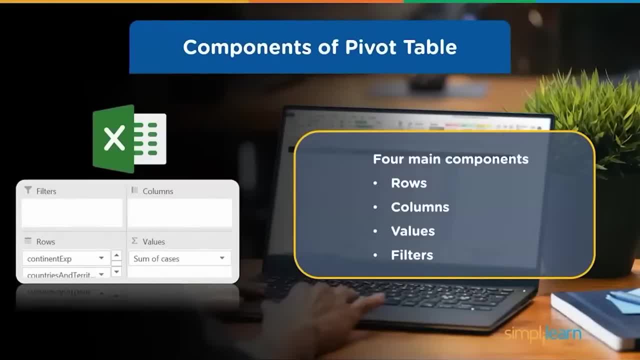 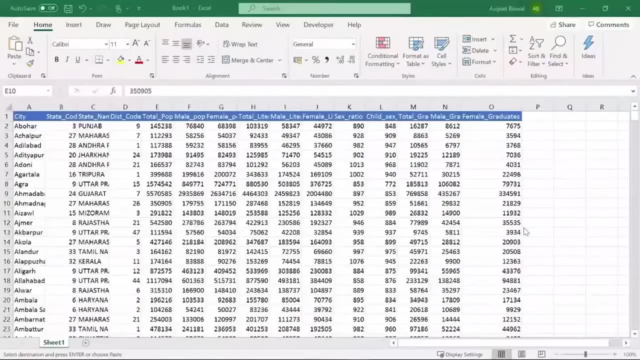 and displays the summarized information. the most common values are sum, average, minimum and maximum. finally, we have filters. filters apply a calculation or restriction to the entire table. so let's jump over to microsoft excel and let me show you the data set that we will use in this demo. 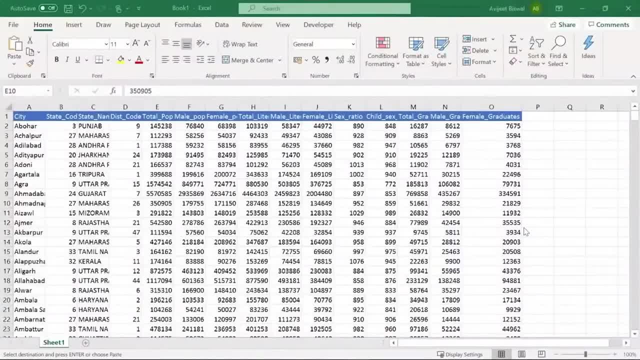 with india being ready for its 16th census in 2021, that is, next year- it is a good time for us to analyze india's last census data from 2011 and see where different states and cities across india stood in terms of population literacy and other socioeconomic 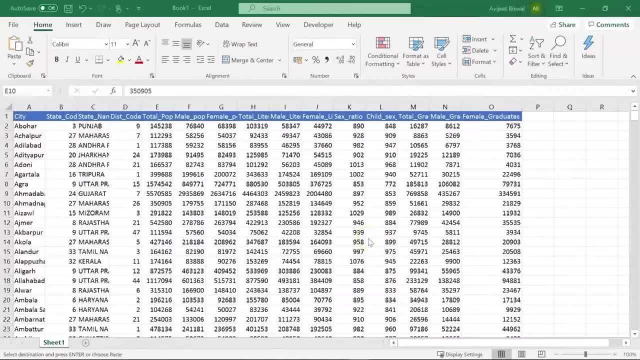 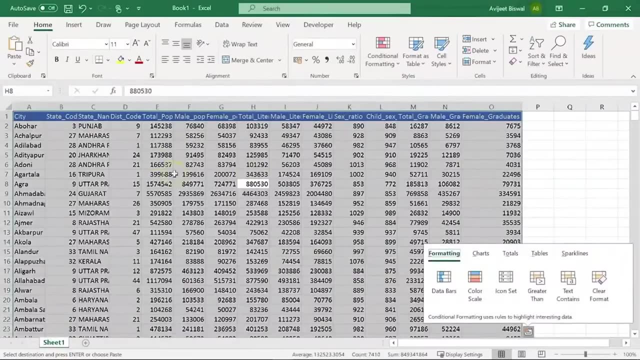 factors. we will analyze this data by creating different pivot tables in excel and explore some of its features. so let's begin first. i will show you one of the features that excel offers us. so suppose i click on any cell and hit control plus q, you can see our entire table. 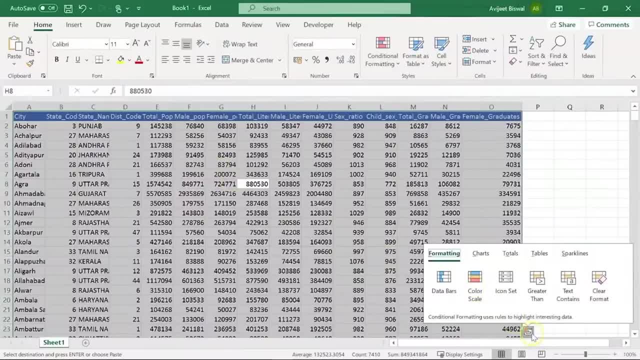 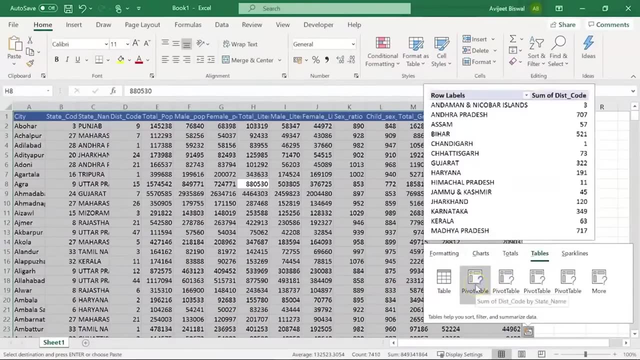 is selected and at the right bottom there is an option of quick analysis. now you can see, by default excel has prompted certain features such as formatting. we have charts, totals and there is one more called tables. now excel by default has created some pivot tables for us. now the first one: 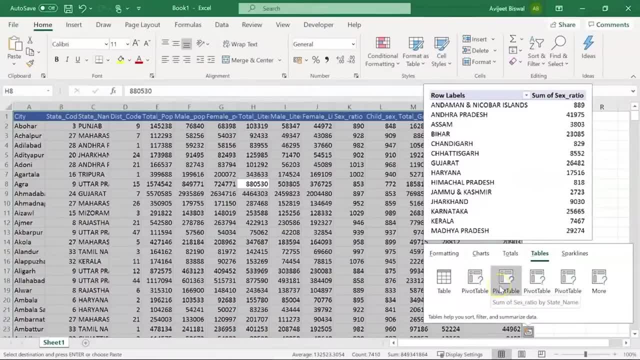 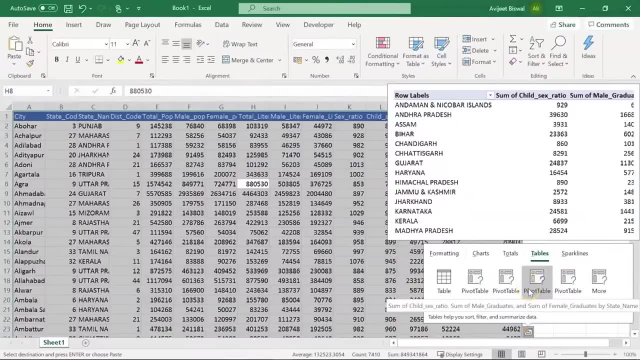 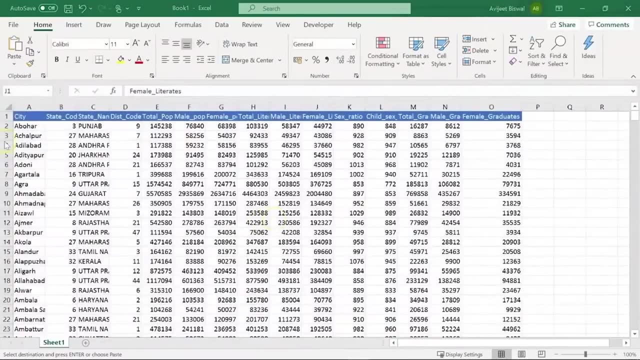 one you see is sum of district code by state names. next we have sum of sex ratio by state name, then we have sum of child sex ratio, sum of male graduates and sum of female graduates by state name, and there are others before creating our pivot table. so let's have a final. 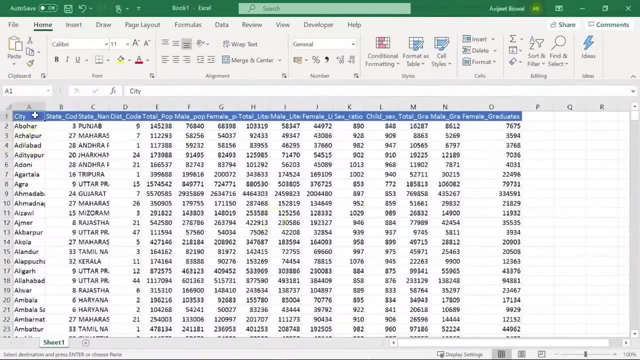 look at our data set. so first column you see is the city column. so there are different cities from different parts of india. then we have the state code. we have the state name, district code, we have the total population, followed by male and female population. next you can see, we have the total. 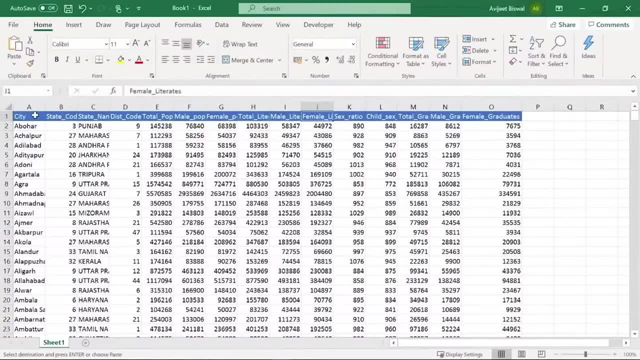 literates from each city, then we have the male and female literates, next we have the sex ratio, then we have the child sex ratio, next we have total number of graduates and finally, you can see, we have male and female graduates. so, using this table, we'll create several. 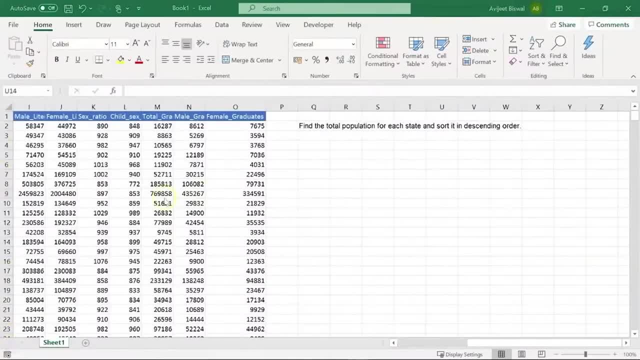 pivot tables. now, first of all, let's create a pivot table to find the total population for each state and sort it in descending order. so you can see, here we have the problem statement. so our first pivot table will have the total population for each of the states in descending order. 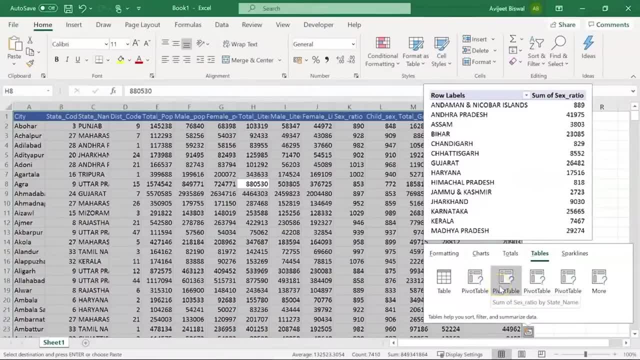 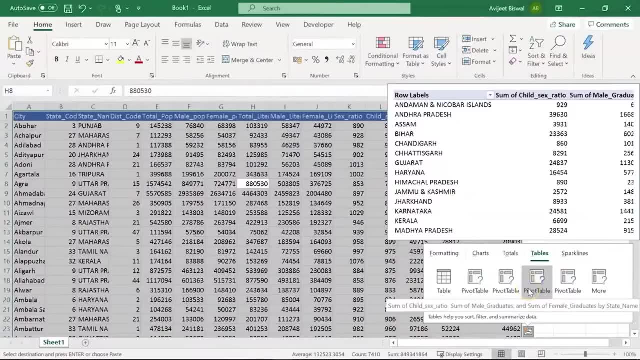 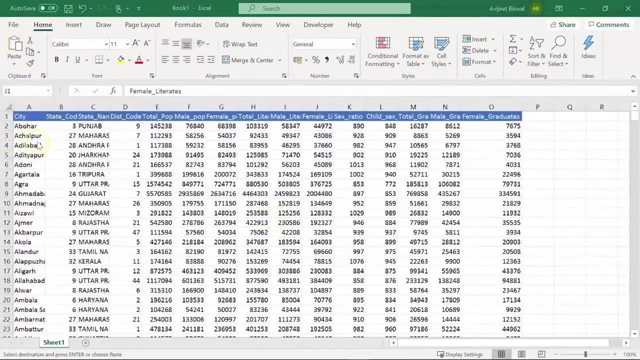 you see, is sum of district code by state names. next we have sum of sex ratio by state name, then we have sum of child sex ratio, sum of male graduates and sum of female graduates by state name, and there are others before creating our pivot table. so let's have a final look at. 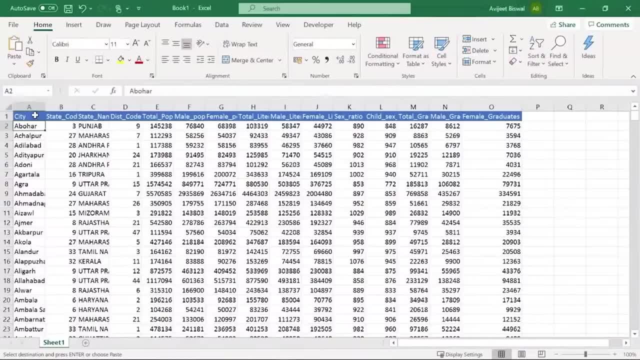 our data set. so first, call column. you see, is the city column. so there are different cities from different parts of india. then we have the state code. we have the state name, district code, we have the total population, followed by male and female population. next you can see: 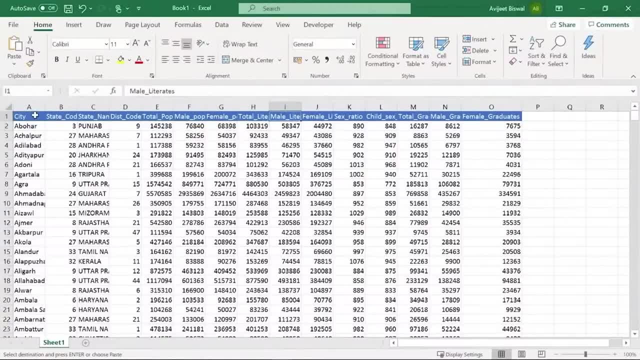 we have the total literates from each city, then we have the male and female literates, next we have the sex ratio, then we have the child sex ratio, next we have total number of graduates and finally, you can see, we have male and female graduates. so, using this table, 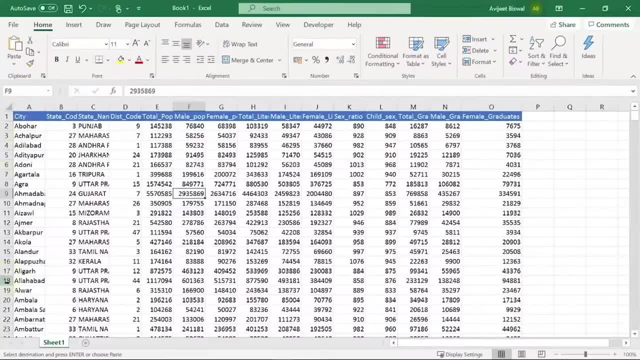 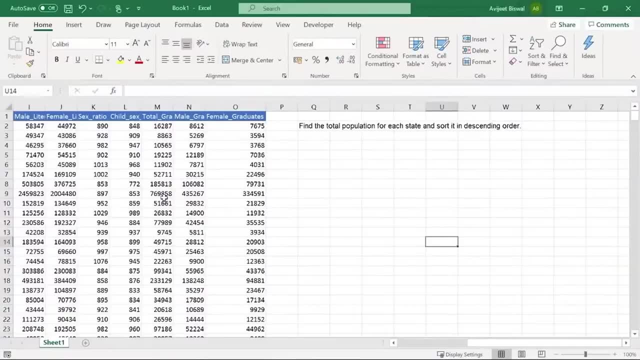 we will create several pivot tables. now, first of all, let's create a pivot table to find the total population for each state and sort it in descending order. so you can see here we have the problem statement. so our first pivot table will have the total population for each of the 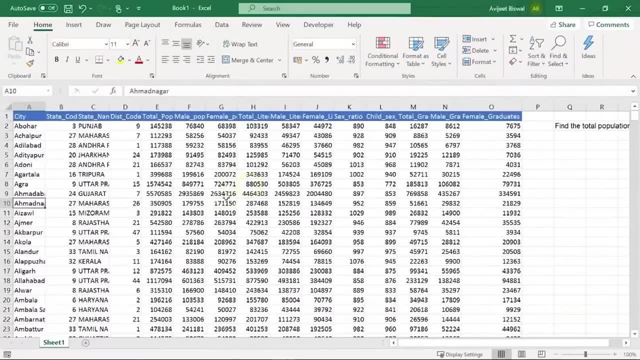 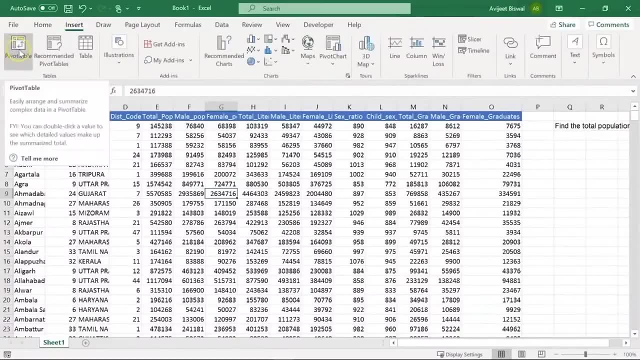 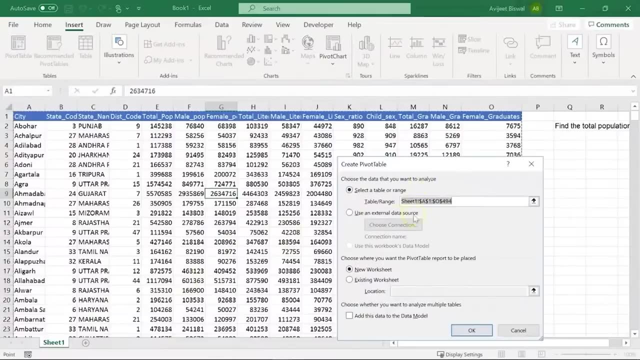 states in descending order. so to create a pivot table, you can click any cell in your data, go to the insert tab and here left you can see we have the option to create a pivot table. so let me select pivot table. now my range is already selected: the entire table. 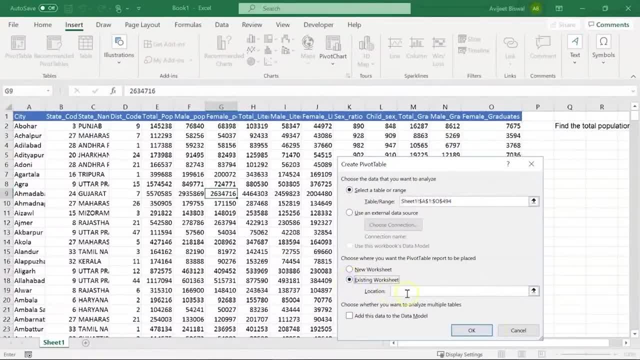 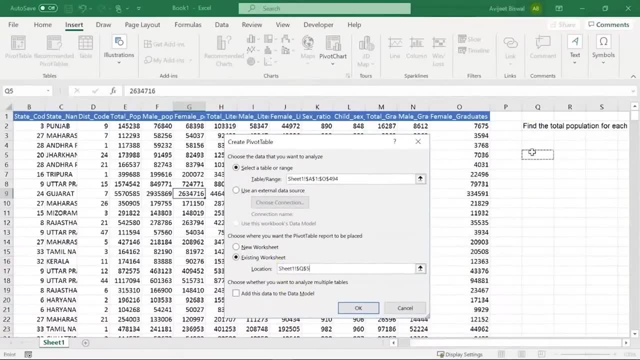 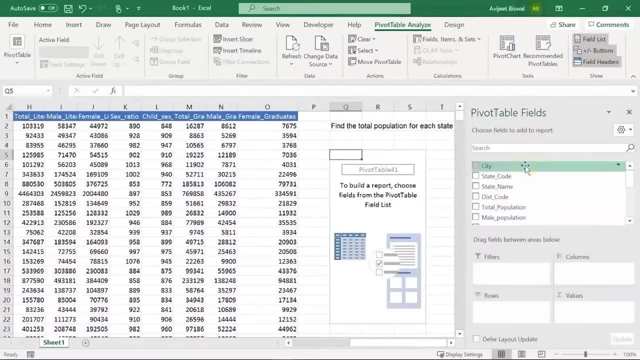 and here i will choose existing worksheet because i want to place my pivot table in the same worksheet and i will give my location. i will point to cell q5. now let me click. ok, you can see the pivot table fields appears here on the right now, since we want to find the total population. 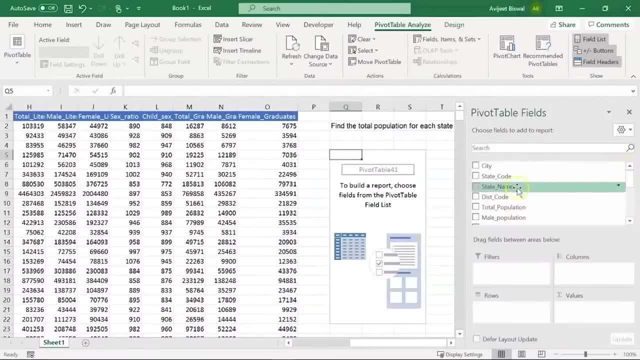 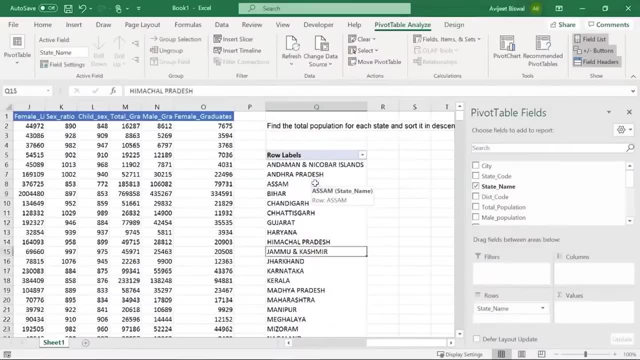 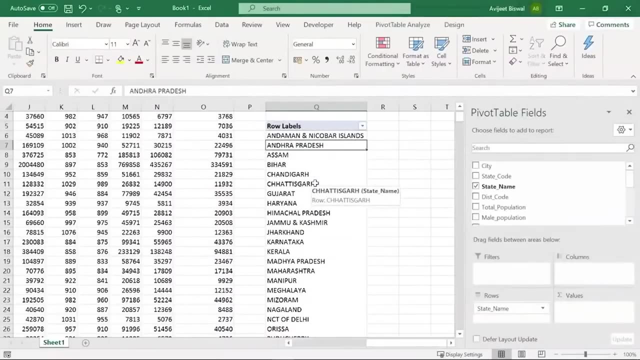 for each state. so what i will do is i will drag my state name onto rows. so here in our pivot table you can see we have the different state names listed. now we want the total population for each of these states, so in the field list i will search for. 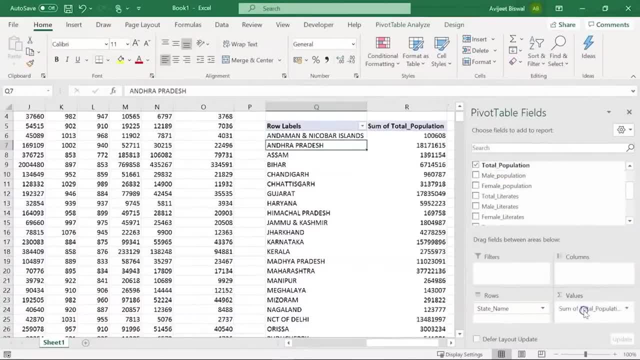 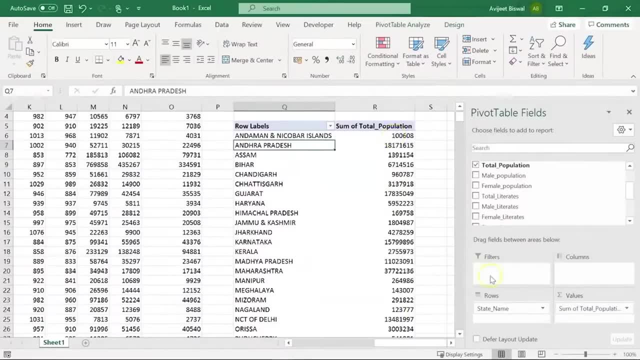 total population, which is this one, and drag it under values. you can see we have our sum of total population for each of these states. by default, excel will sum any numeric column. you can always change it to average, minimum, maximum, anything you want. now we want to sort this column in. 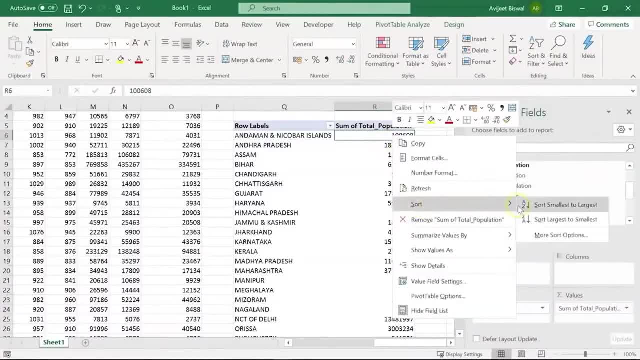 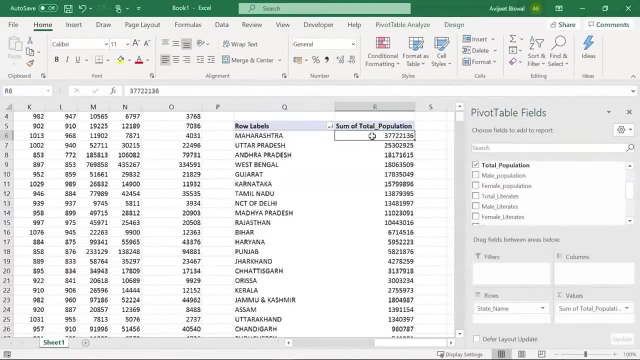 descending order. so i right click, go to sort option and choose z to a. that is largest to smallest. you can see here: in 2011 Maharashtra had the highest number of population, or the total population in Maharashtra was the highest. then it was Uttar Pradesh we had 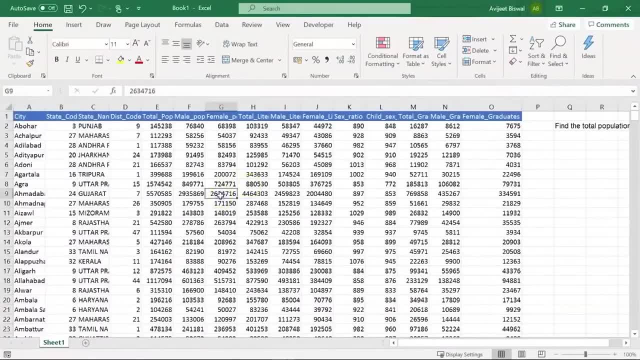 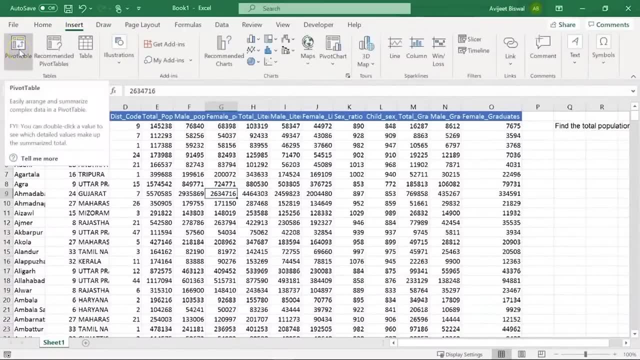 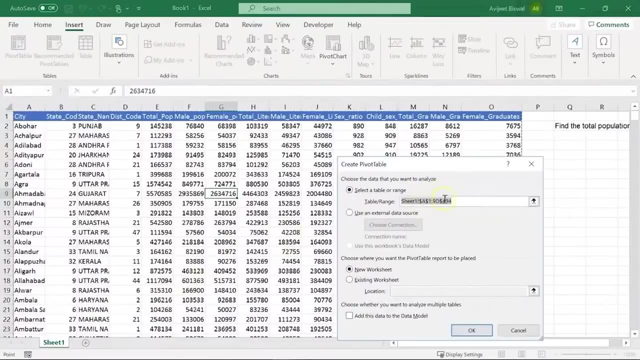 so to create a pivot table, you can click any cell in your data, go to the insert tab and here left you can see we have the option to create a pivot table. so let me select pivot table. now my range is already selected- the entire table, and here i will. 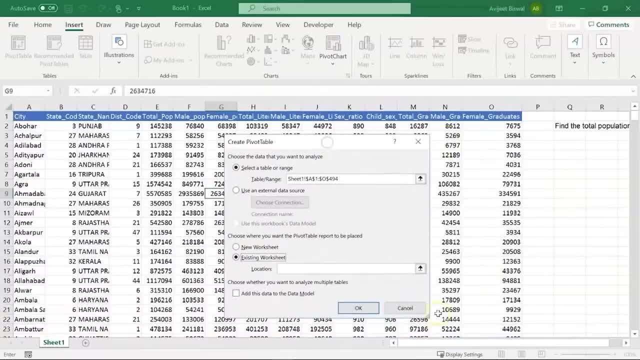 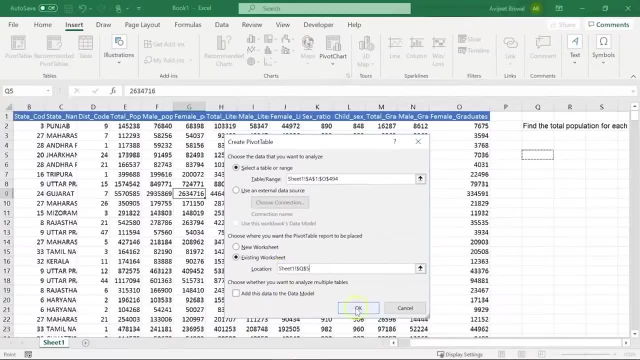 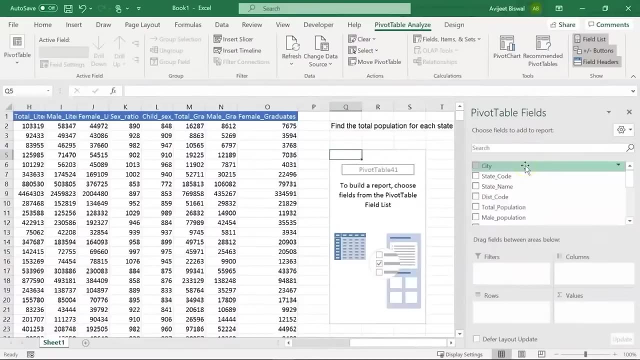 choose existing worksheet because i want to place my pivot table in the same worksheet and i'll give my location. i'll point to cell q5. now let me click. ok, you can see the pivot table fields appears here on the right now. since we want to find the total, 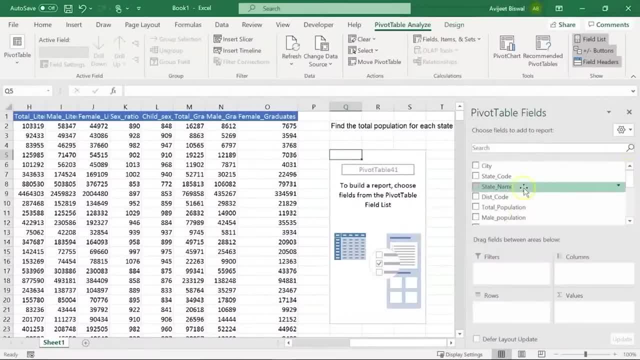 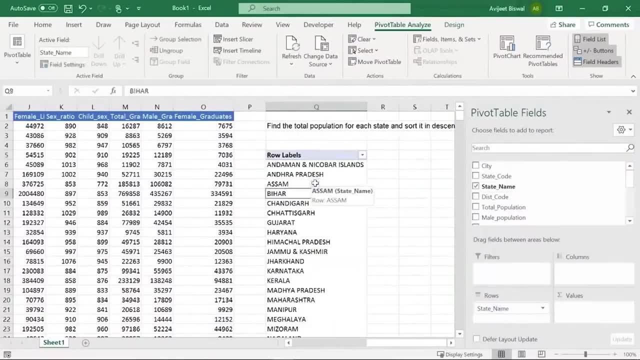 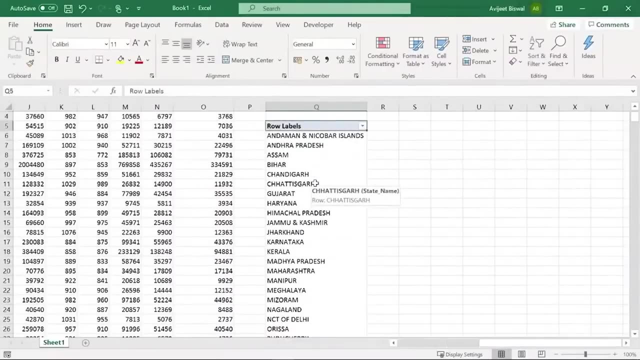 population for each state. so what i'll do is i'll drag my state name onto rows. so here in our pivot table you can see we have the different state names listed. now we want the total population for each of these states, so in the field list i'll search. 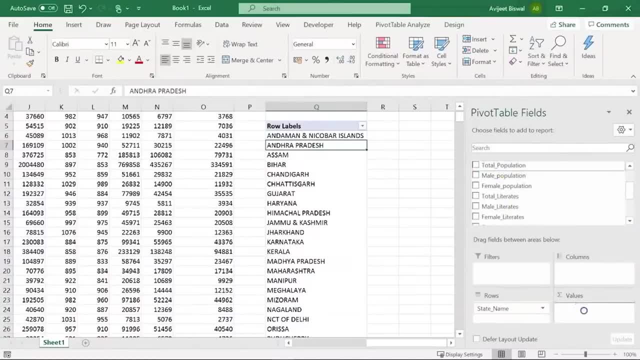 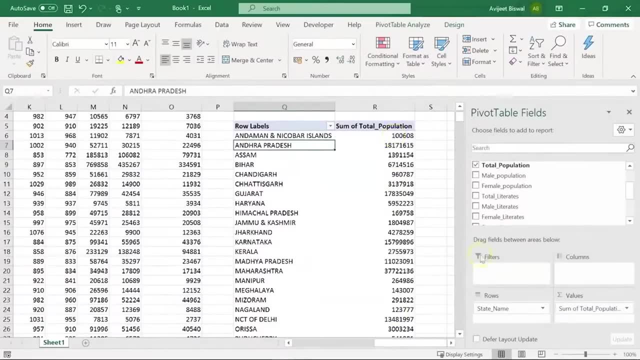 for total population, which is this one, and drag it under values. you can see we have our sum of total population for each of these states. by default, excel will sum any numeric column. you can always change it to average, minimum, maximum, anything you want. now we want to sort this column. 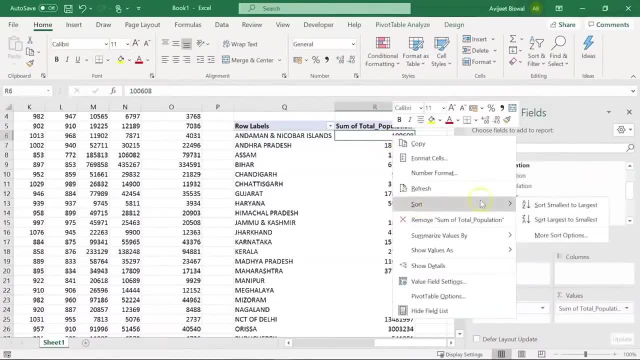 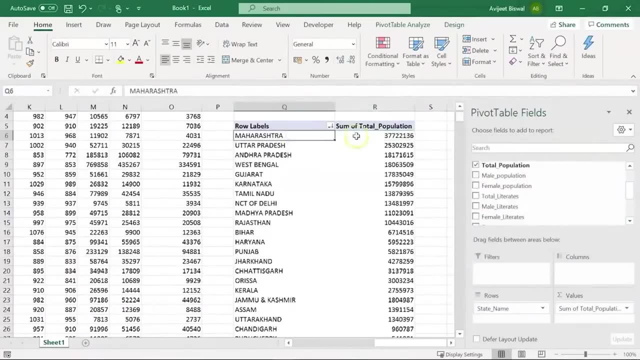 in descending order. so i right click, go to sort option and choose z to a. that is largest to smallest. you can see here in 2011 maharashtra had the highest number of population, or the total population in maharashtra was the highest. then it was uttar pradesh. 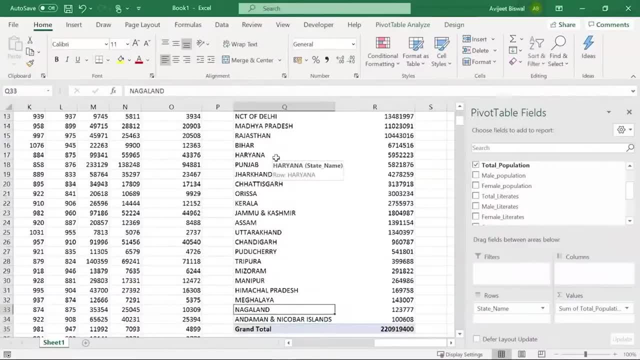 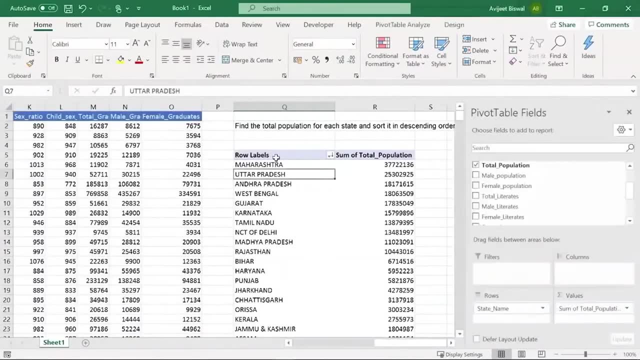 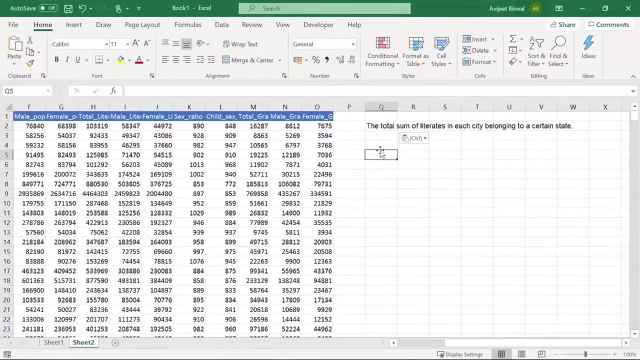 we had andhra pradesh and if i come down, we have nagaland and andaman and nicobar islands towards the end. so this is a simple pivot table that we created. now the next problem we have is we want to find the total sum of literates in each city belonging. 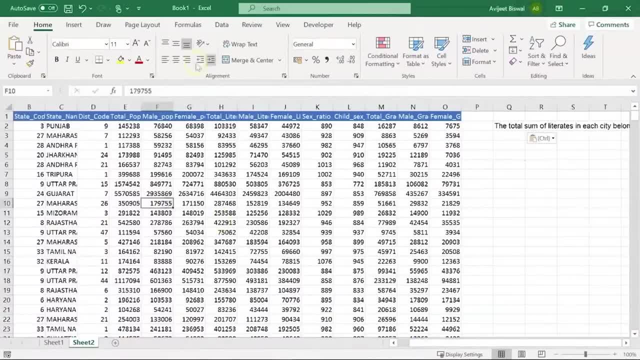 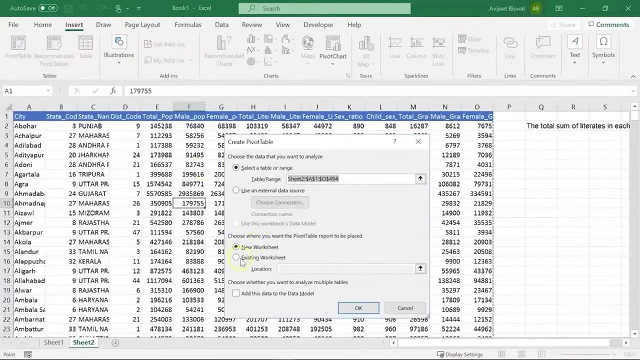 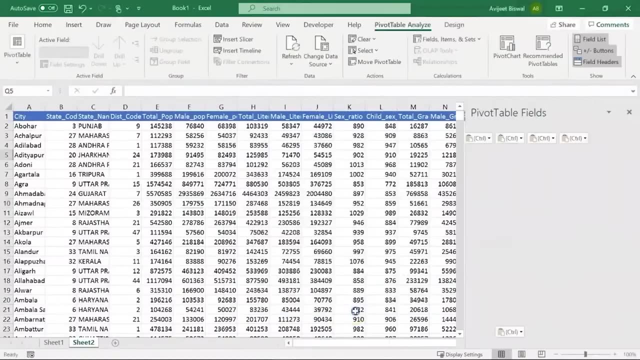 to a certain state. so let's see how to do it. i'll click on any cell, go to insert and here i can click on pivot table. my range is selected. i'll choose existing worksheet and give my location, which is q5. i click on ok, now here. 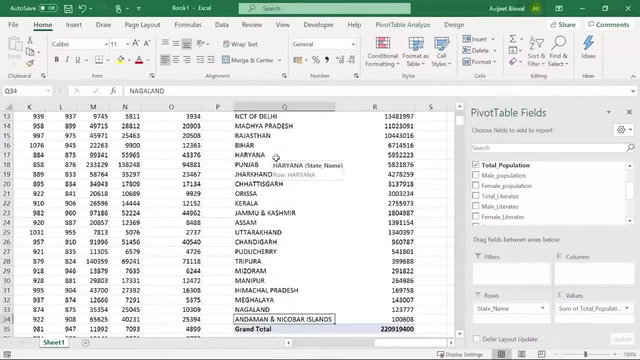 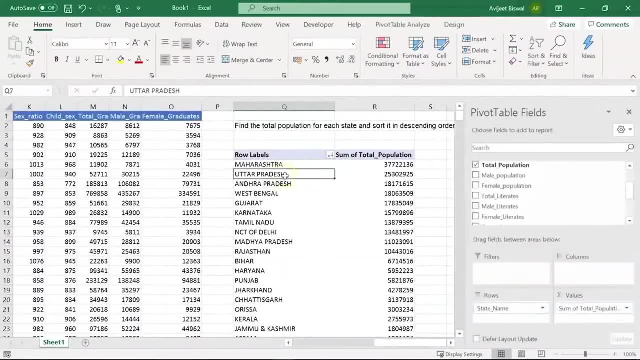 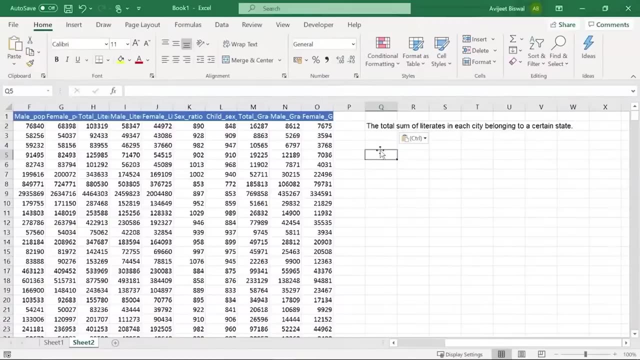 Andhra Pradesh and if i come down, we have Nagaland and Andaman and Nicobar islands towards the end. so this is a simple pivot table that we created. now the next problem we have is we want to find the total sum of literates in each city belonging to. 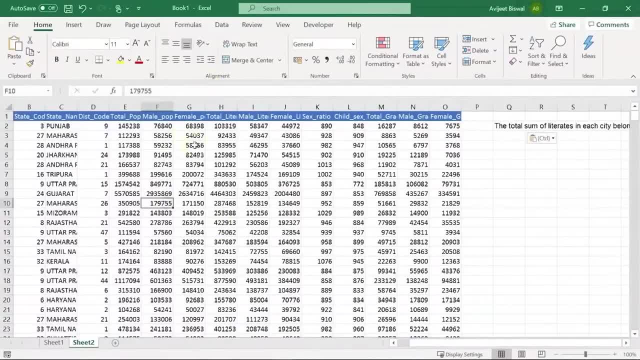 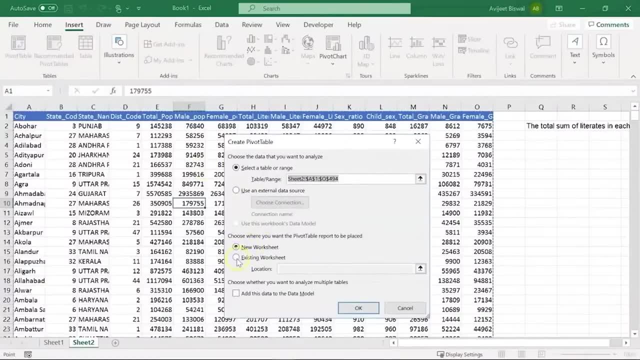 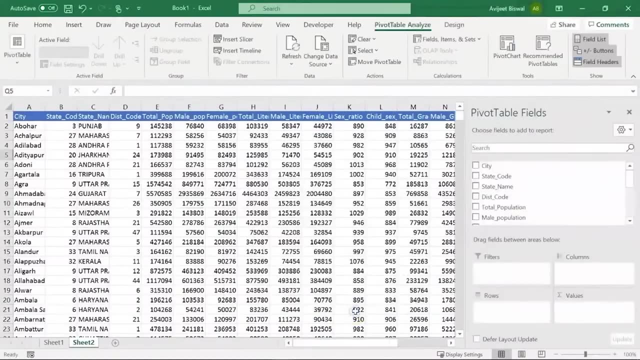 a certain state. so let's see how to do it. i will click on any cell, go to insert and here i can click on pivot table. my range is selected. i will choose existing worksheet and give my location, which is q5. i click on ok, now here. 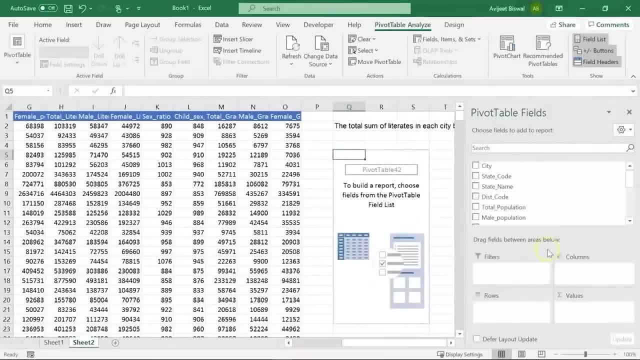 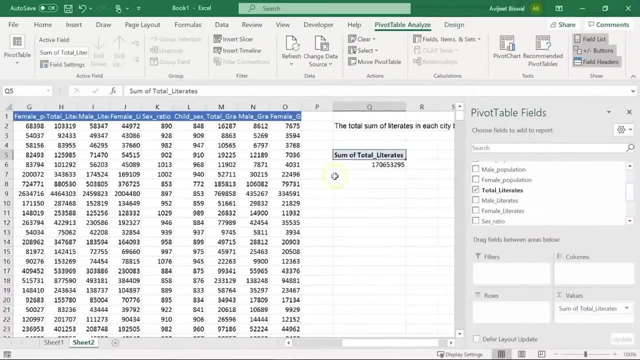 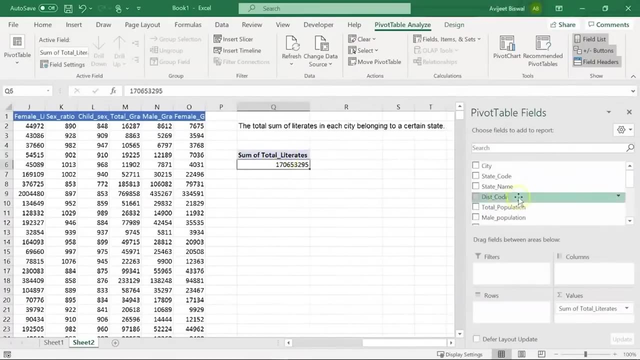 we want to find the total sum of literates. so what i'll do is first let me drag total literates column to values. you have the total sum of literates from all the states. next, i want to see the sum of total literates based on: 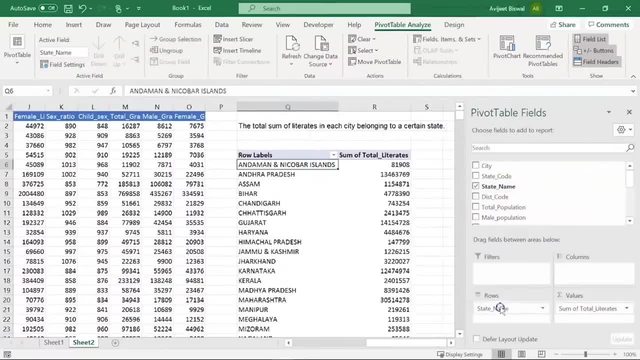 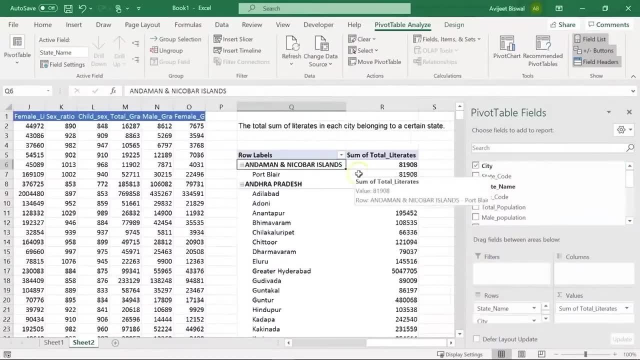 states and cities. so let me first drag state name onto rows and then we'll drag city onto rows. you can see, here we have our pivot table ready. to the left of the pivot table, you can see, we have the state names and the cities per state and on 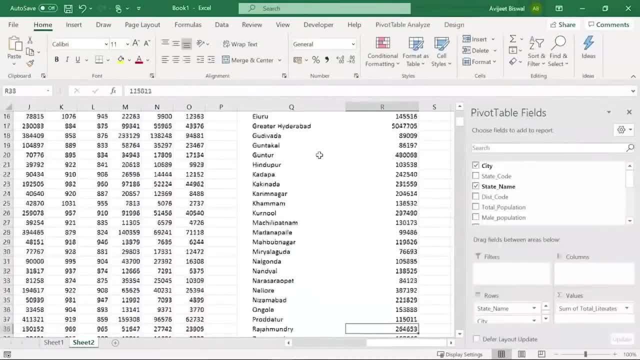 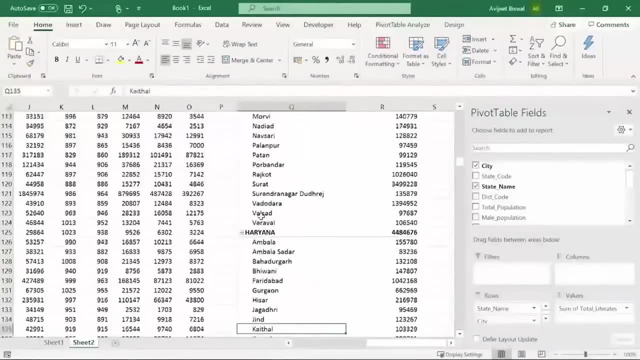 the right, you can see the total number of literates from each city. if i scroll down, we have Assam, then you can see we have Bihar, and if i keep scrolling, we have all the states: Haryana, Himachal Pradesh, that's, Jammu and Kashmir, which has now become a 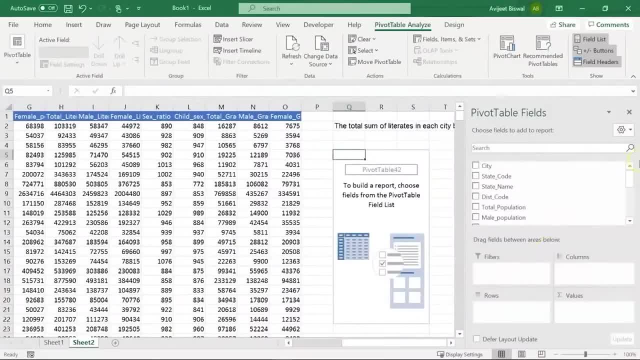 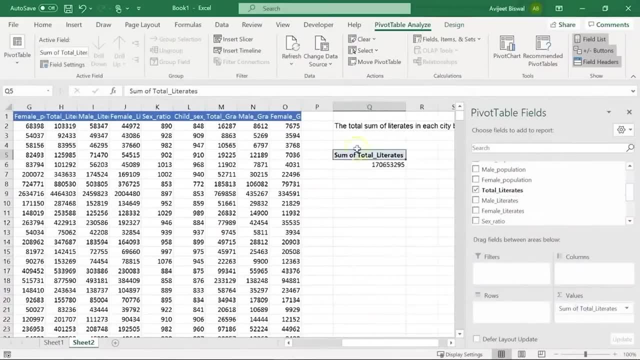 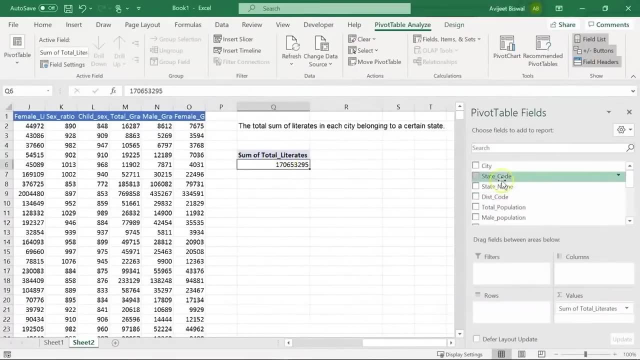 we want to find the total sum of literates. so what i will do is first let me drag total literates column to values. you have the total sum of literates from all the states. next, i want to see the sum of total literates based on: 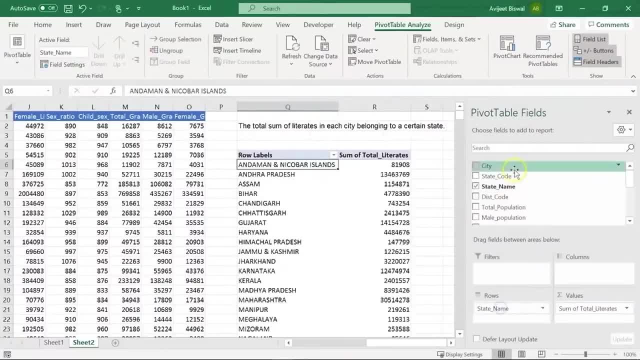 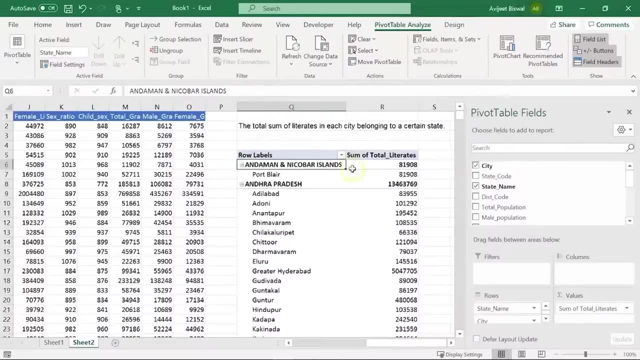 states and cities. so let me first drag state name onto rows and then we will drag city onto rows. you can see, here we have our pivot table ready. to the left of the pivot table, you can see, we have the state names and the cities per state, and on the right 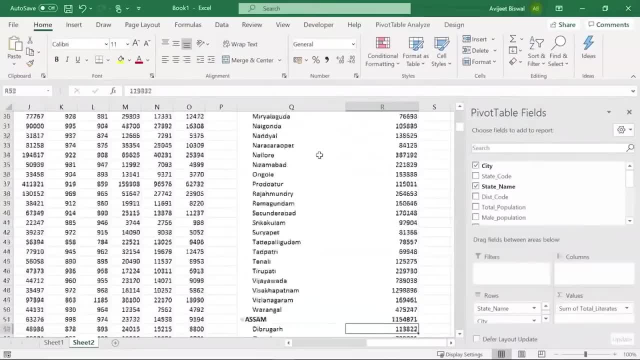 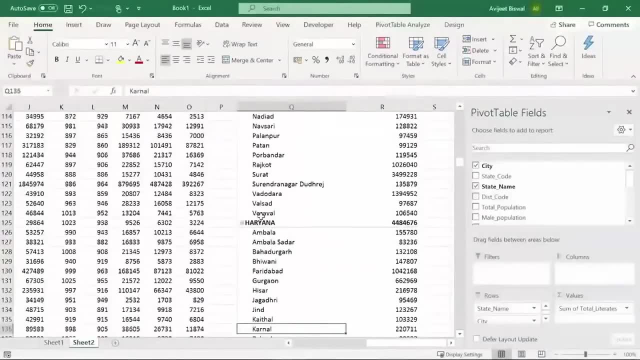 you can see the total number of literates from each city. if i scroll down, we have Assam, then you can see we have Bihar, and if i keep scrolling we have all the states: Haryana, Himachal Pradesh, that's Jammu and Kashmir, which has now become a union territory. 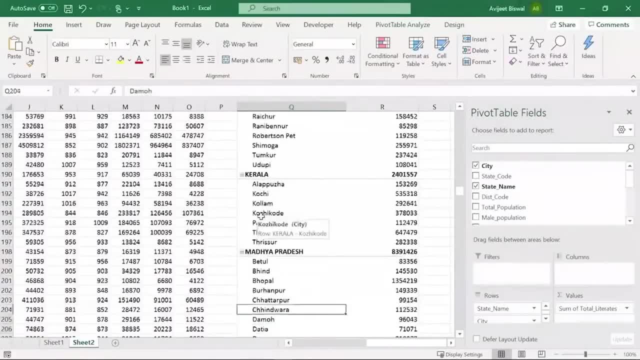 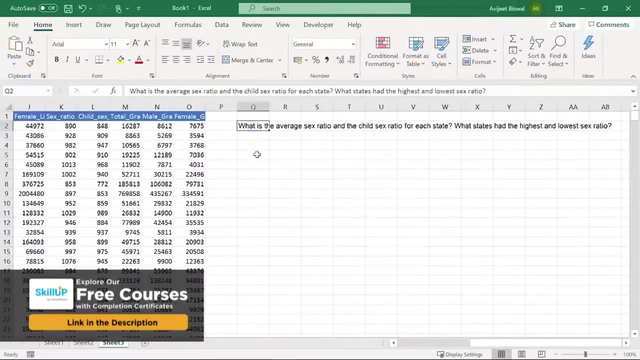 we have Jharkhand, Karnataka and other states as well, moving on. ok, so the next thing we want to see is what is the average sex ratio and the child sex ratio for each state? with that, we also want to find the states that had the highest and lowest. 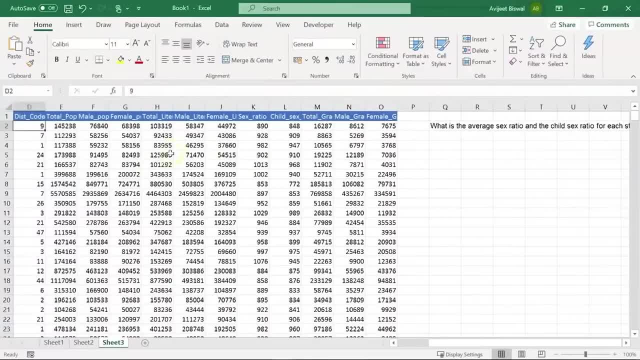 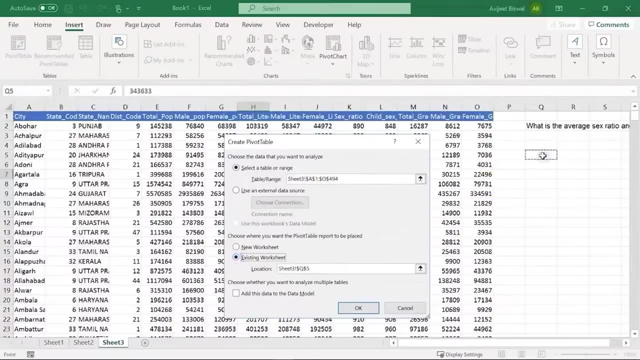 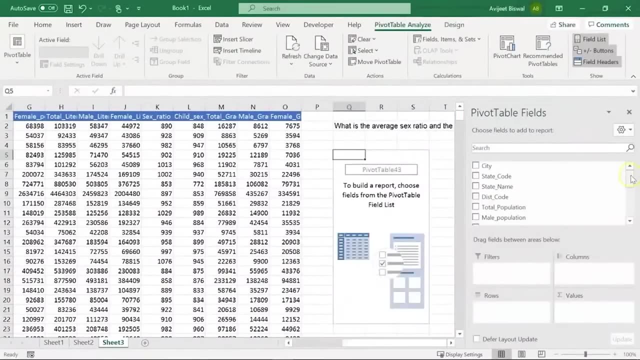 sex ratio in 2011. so let's create a pivot table for this. i'll click on any cell. go to insert. choose pivot table. click on existing worksheet. i'll select cell Q5 and click on ok. now, since we want the average sex ratio and the 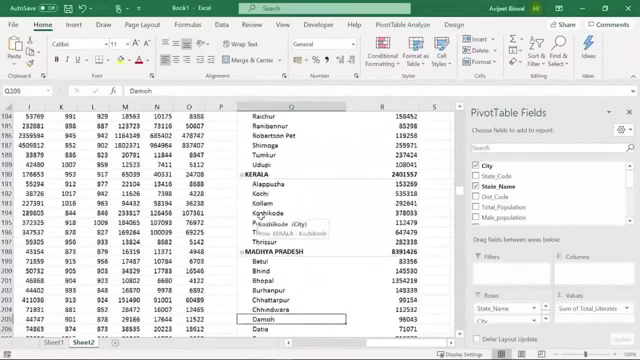 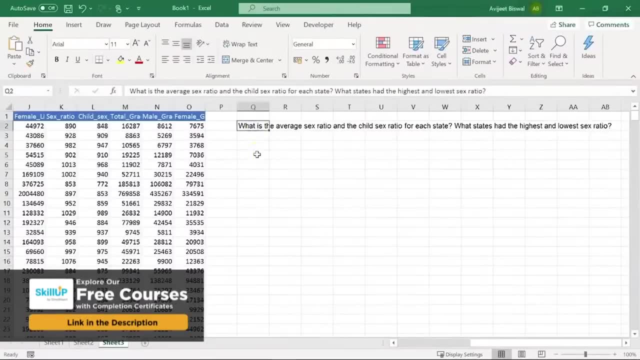 union territory. we have Jharkhand, Karnataka and other states as well, moving on. ok, so the next thing we want to see is what is the average sex ratio and the child sex ratio for each state. with that, we also want to find the states that had the highest. 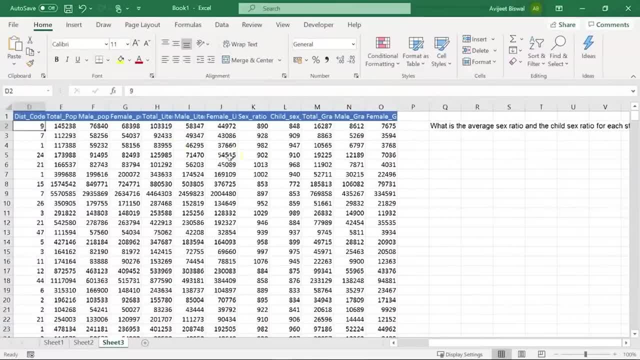 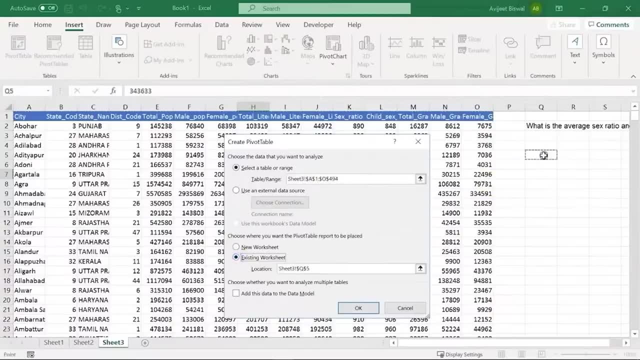 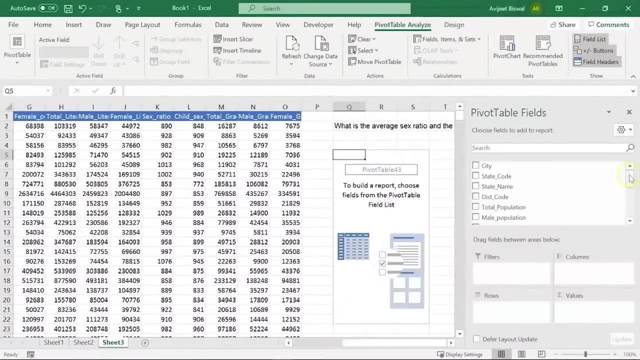 and lowest sex ratio in 2011. so let's create a pivot table for this. i'll click on any cell. go to insert. choose pivot table. click on existing worksheet. i'll select cell Q5 and click on ok. now, since we want the average sex ratio, 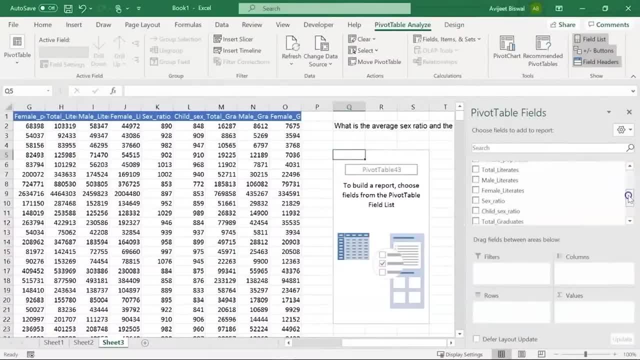 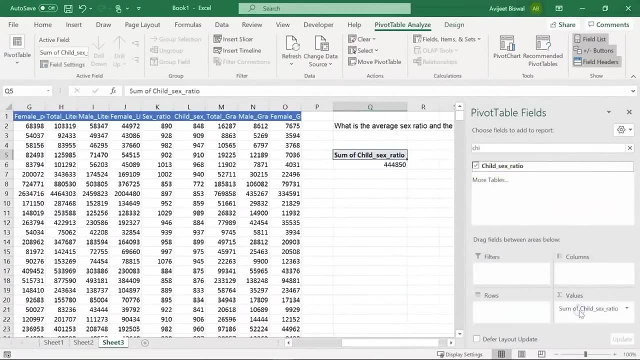 and the child sex ratio. so first i'll drag those columns. either you can manually scroll and drag it or here you have the option to search for it. so if i look for child you can see we have the same column listed. you can just drag it from there. 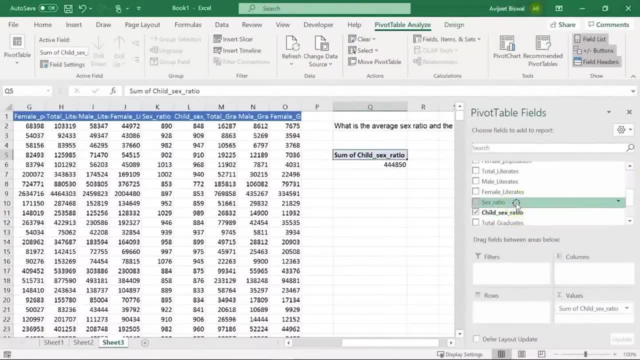 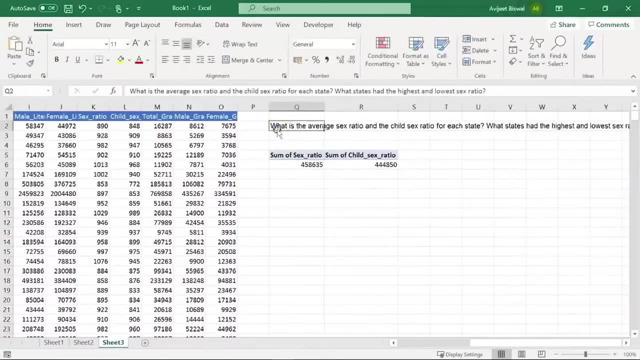 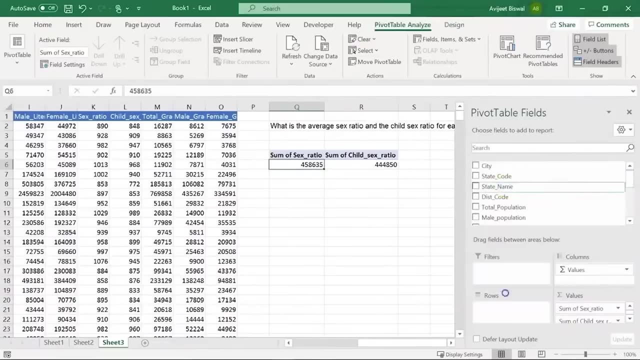 let me delete this, and i also want the sex ratio, so i'll place it on top of child sex ratio. next, we want to see it based on different states, so what i'll do is i'll take state name and put it under rows. so here you can see, we have our. 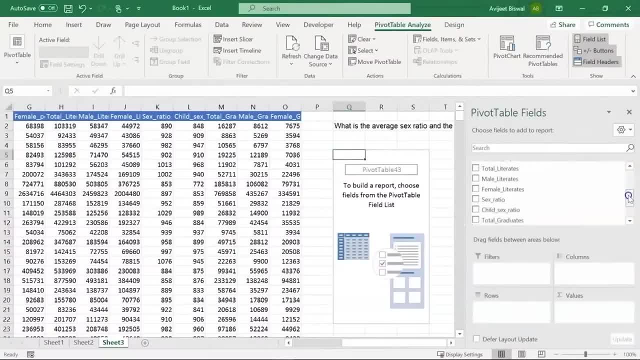 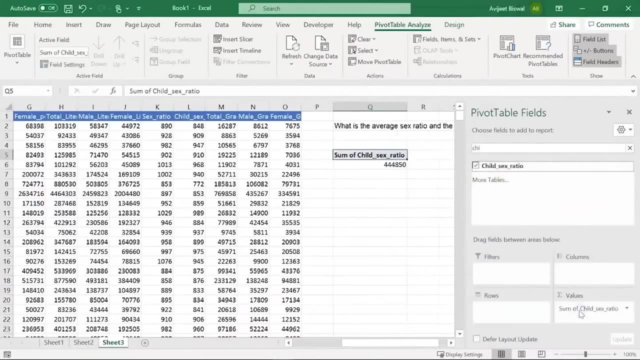 child sex ratio. so first i'll drag those columns. either you can manually scroll and drag it or here you have the option to search for it. so if i look for child you can see we have the same column listed. you can just drag it from there. let me delete. 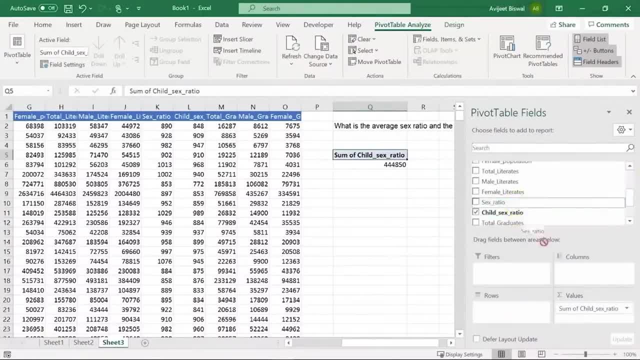 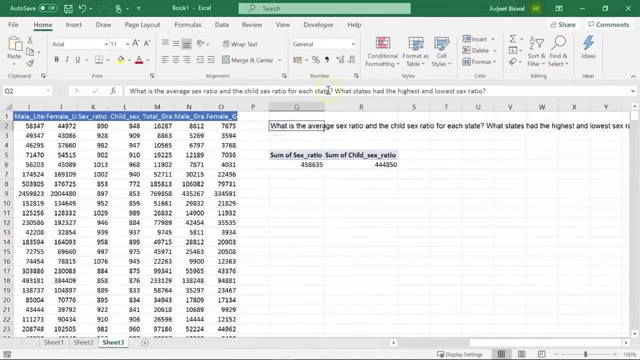 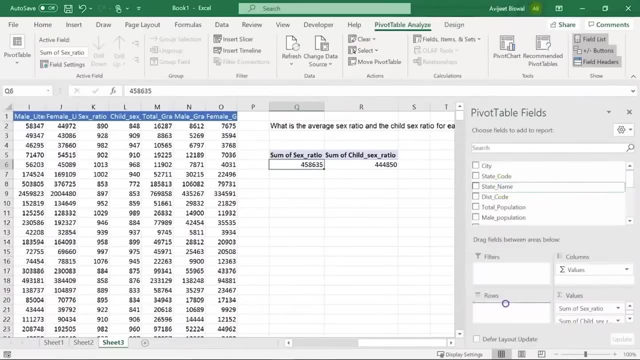 this, and i also want the sex ratio, so i'll place it on top of child sex ratio. next, we want to see it based on different states, so what i'll do is i'll take state name and put it under rows. so here you can see, we have our pivot table. 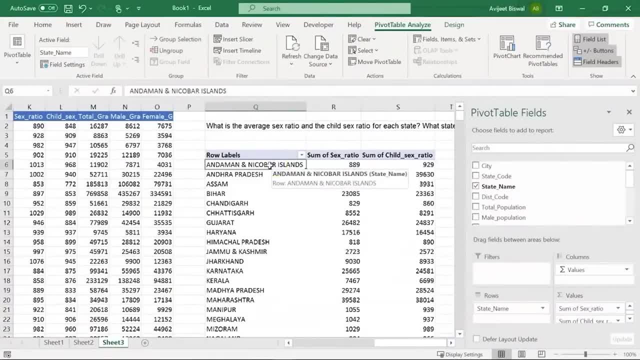 pivot table ready. on the left you can see we have the different state names listed and on the right we have the values. now we want to find the average. now, by default, excel will sum the numeric columns you can see. it tells you sum of sex ratio and child sex ratio. 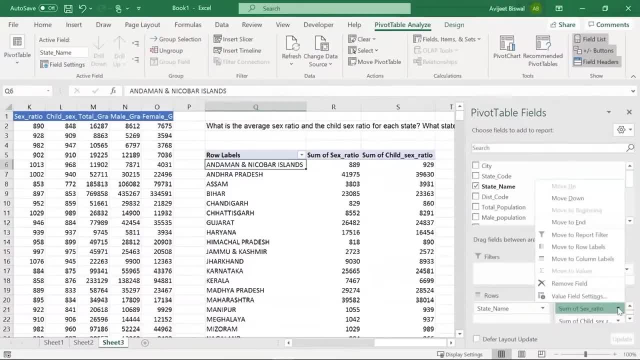 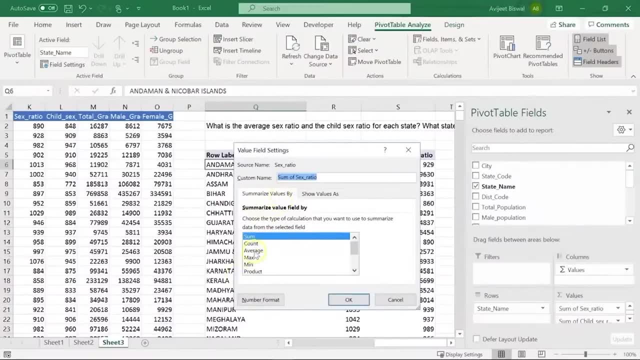 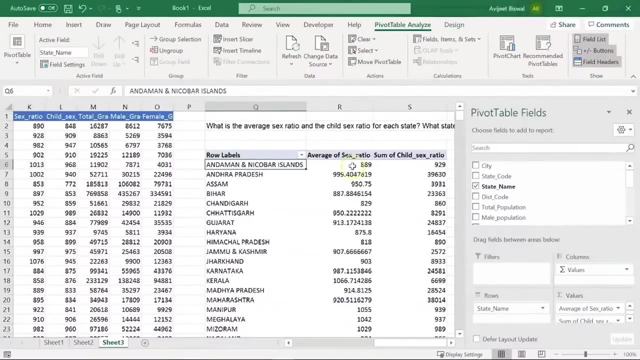 so what you can do: you can click on this drop down and go to value field settings and here summarize values by. you can choose average. you can see the custom name. it says average of sex ratio. click on. ok, our entire column is now giving us the average sex ratio. 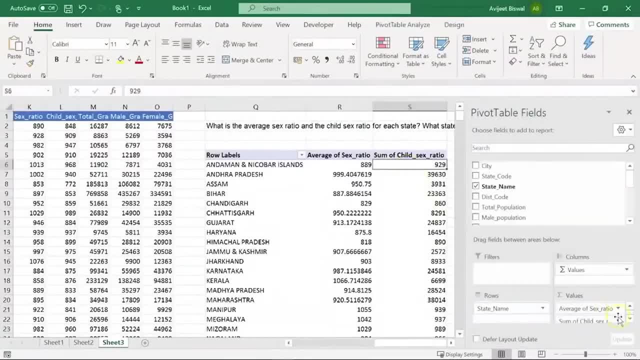 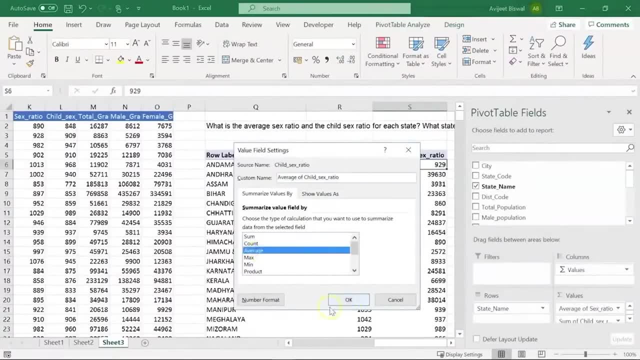 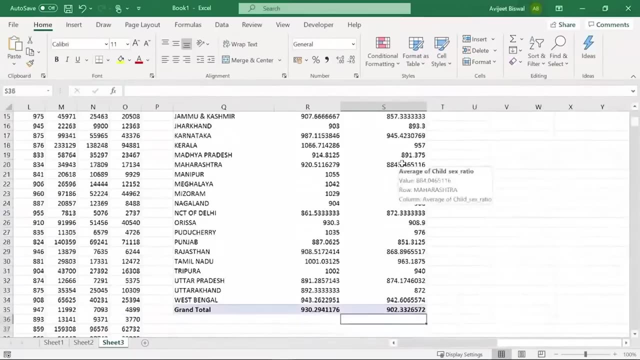 similarly for this column. let me convert it into average. i'll again click on the drop down, go to value field settings, click on average and click ok and you can see. here we have the average of child sex ratio for each of the states. now the next question. 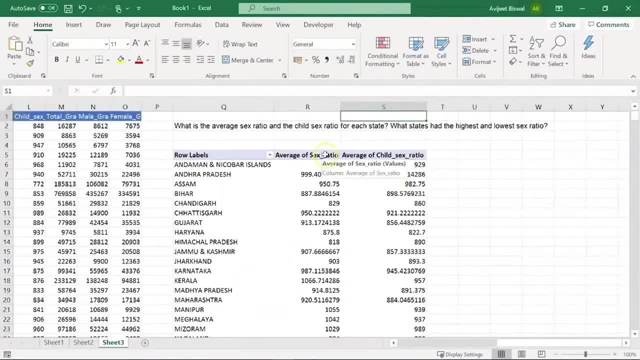 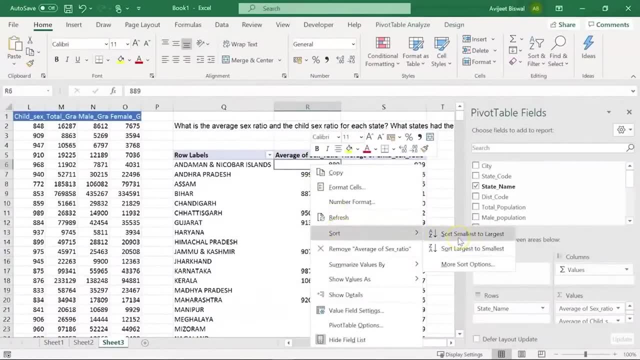 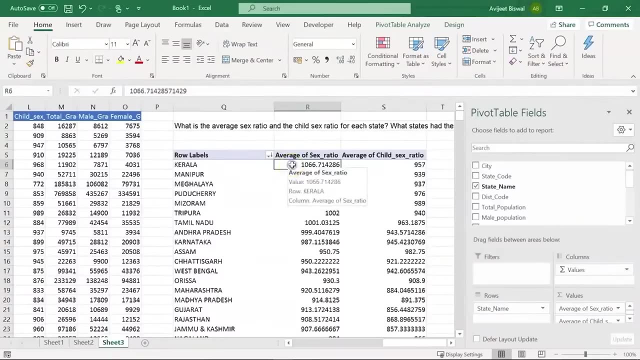 says which states had the highest and lowest sex ratio. so we'll consider this column. so we'll sort it in any order you want. you can do it either ascending or descending. let me sort it in descending order. you can see. we have our column sorted now, so in 2011. 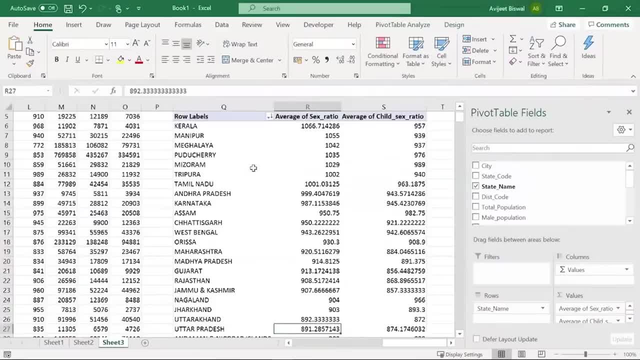 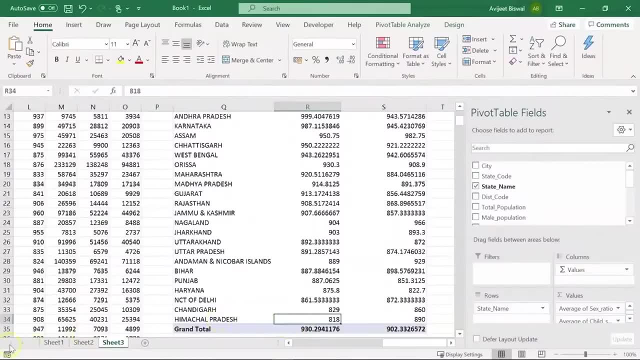 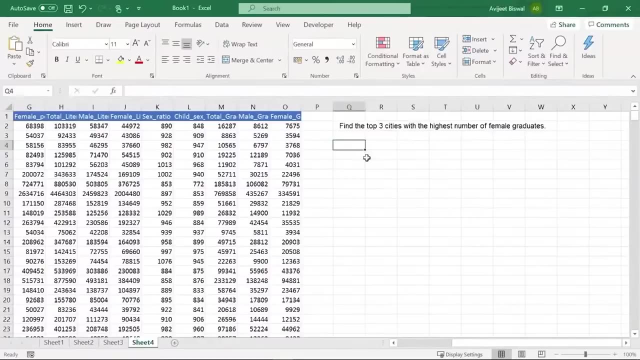 Kerala had the highest sex ratio and if i scroll down to the bottom you can see Himachal Pradesh had the lowest, which is around 818. up next let's explore one more feature of pivot table. suppose you want to see the top or bottom few rows of a pivot table. 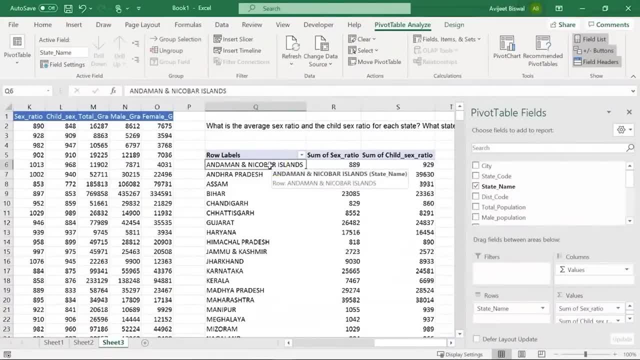 ready. on the left you can see we have the different state names listed and on the right we have the values. now we want to find the average. now, by default, excel will sum the numeric columns you can see. it tells you sum of sex ratio and child sex ratio. so what you? 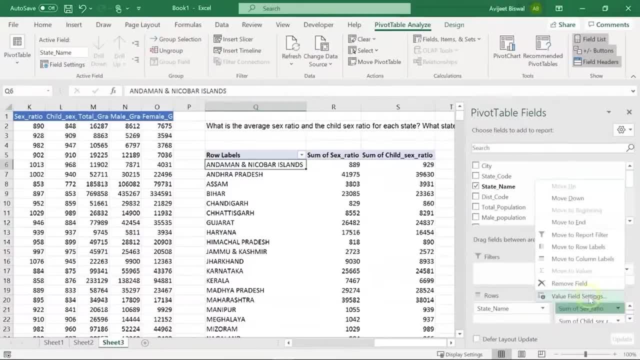 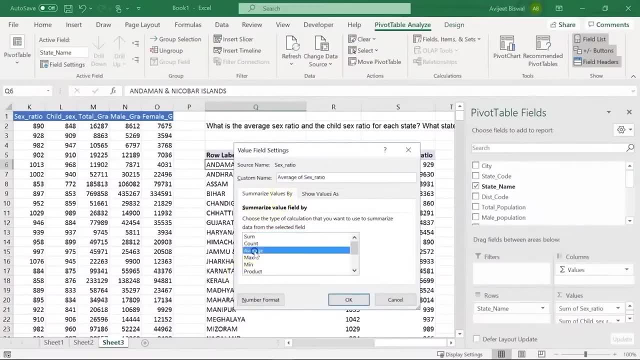 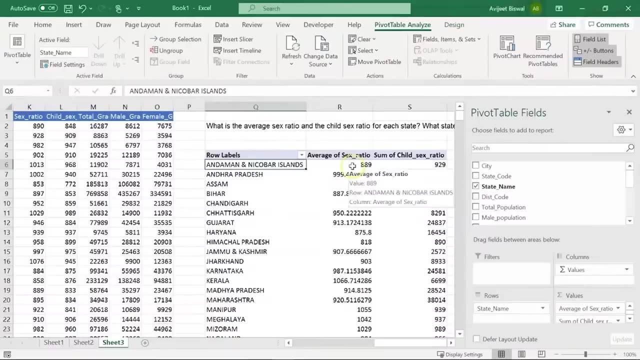 can do. you can click on this drop down and go to value field settings and here summarize values by. you can choose average. you can see the custom name. it says average of sex ratio. click on ok, our entire column is now giving us the average sex ratio. similarly, 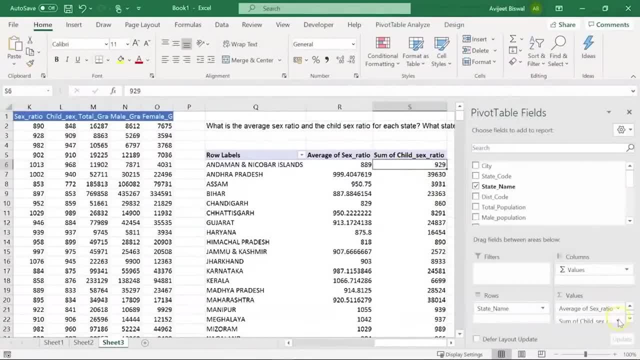 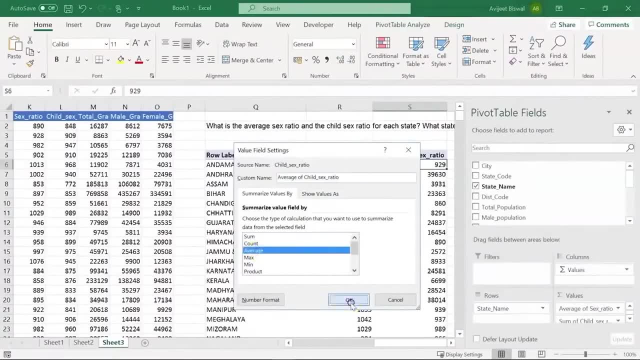 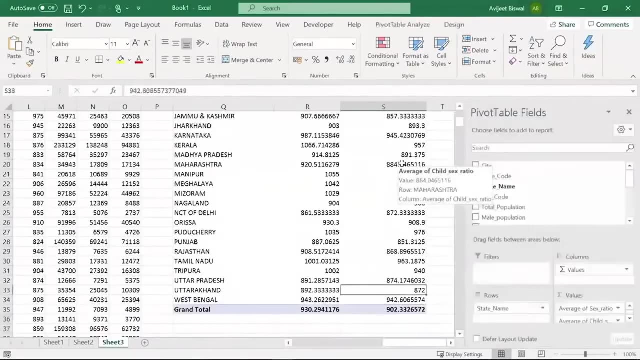 for this column. let me convert it into average. i'll again click on the drop down, go to value field settings, click on average and click ok and you can see. here we have the average of child sex ratio for each of the states. now the next question says: 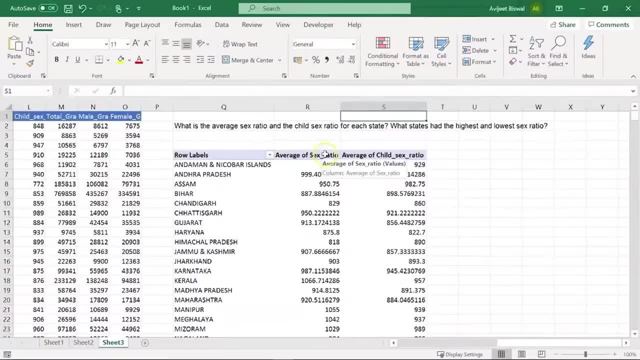 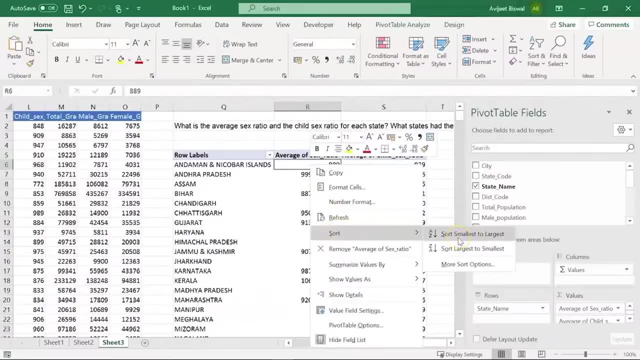 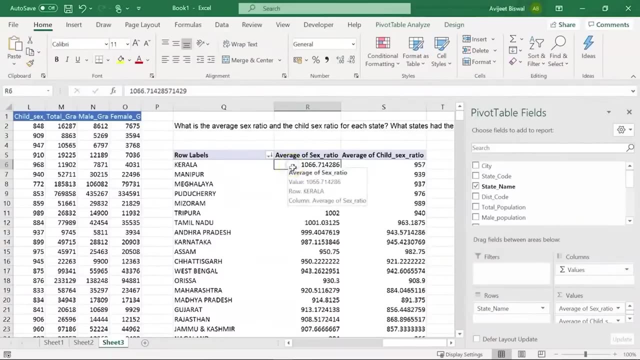 which states had the highest and lowest sex ratio. so we'll consider this column. so we'll sort it in any order you want. you can do it either ascending or descending. let me sort it in descending order. you can see, we have our column sorted now, so in 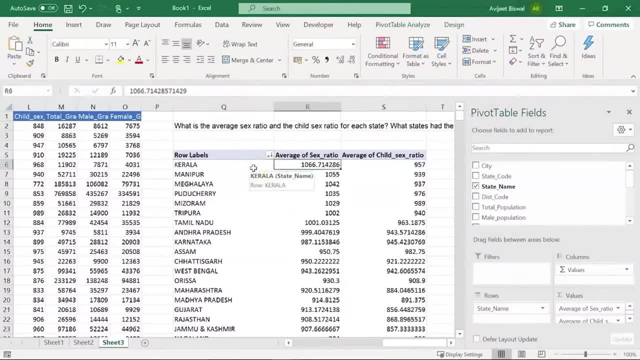 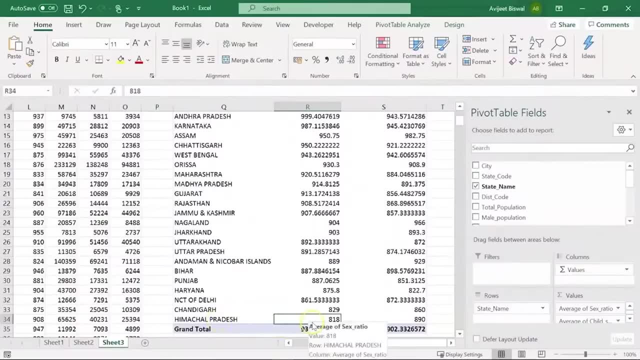 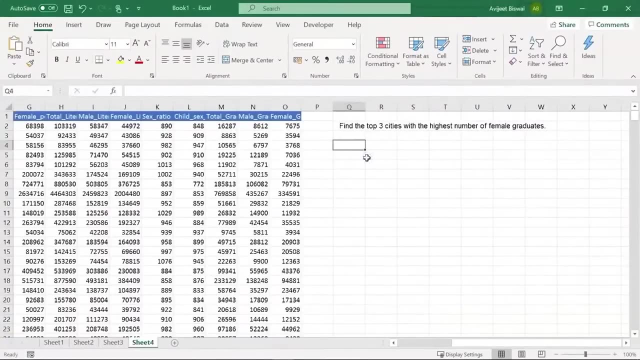 2011, kerala had the highest sex ratio and if i scroll down to the bottom you can see himanchal pradesh had the lowest, which is around 818. up next, let's explore one more feature of pivot table. so suppose you want to see the top or bottom few rows. 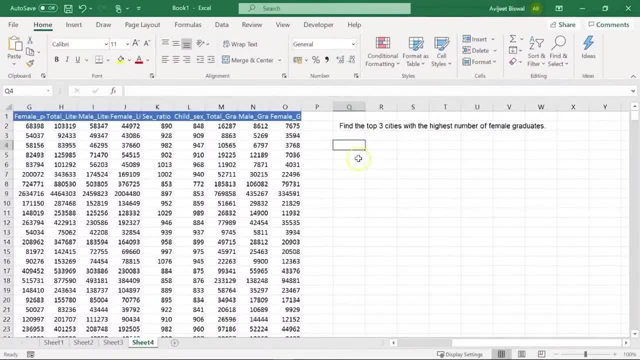 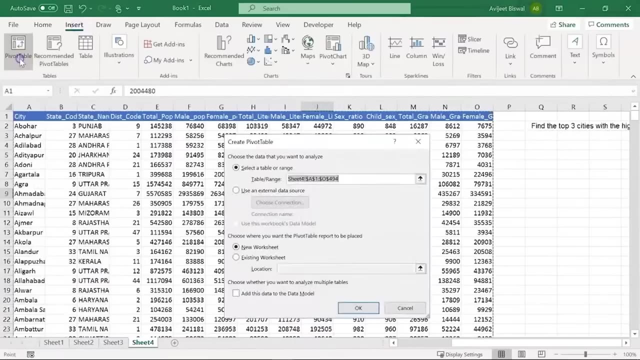 of a pivot table, you can do that as well. so here we have a question at hand. we want to find the top three cities with the highest number of female graduates. so let's see from the entire pivot table how we can filter the top three cities. so i'll go to insert: 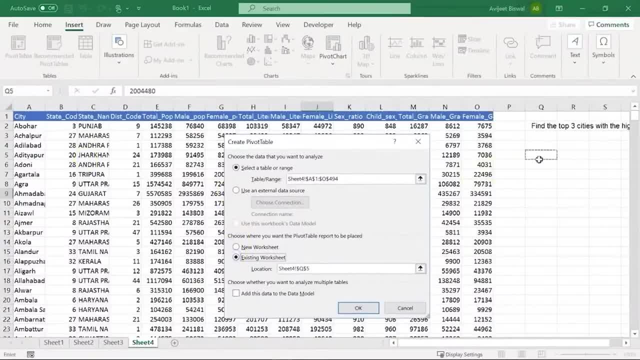 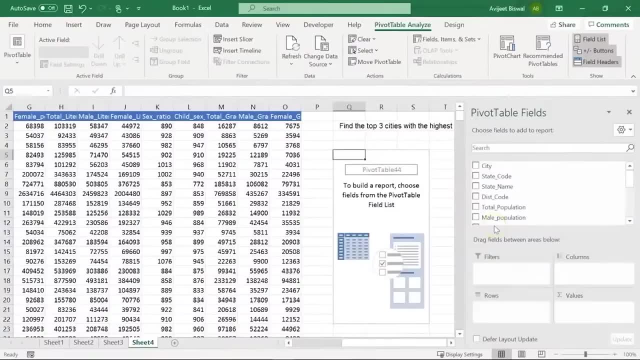 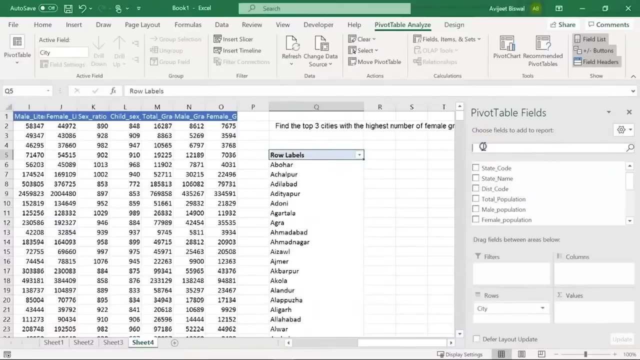 click on the pivot table option, go to existing worksheet, click on q5 and hit ok. now, since we want to find the top three cities, i'll drag city column onto rows. and then we want the female graduates, so in the search bar i'll look for female. 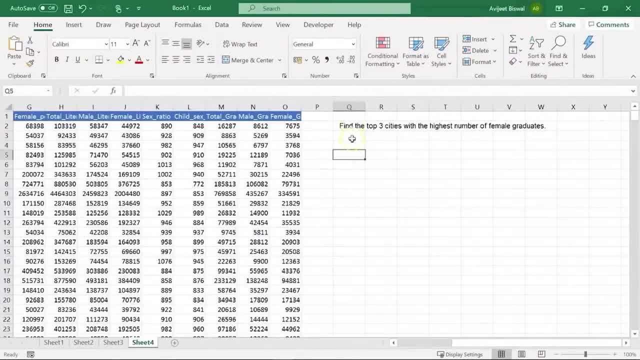 you can do that as well. so here we have a question at hand. we want to find the top three cities with the highest number of female graduates. so let's see from the entire pivot table how we can filter the top three cities. so i'll go to insert: 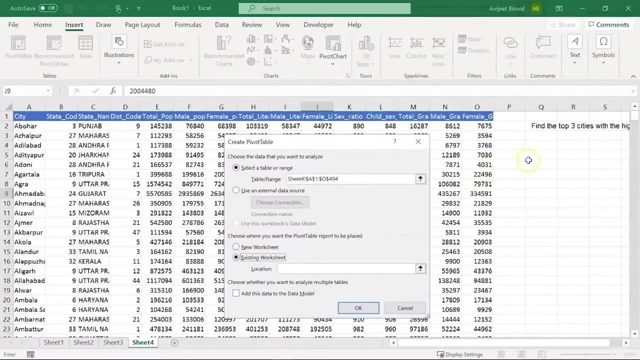 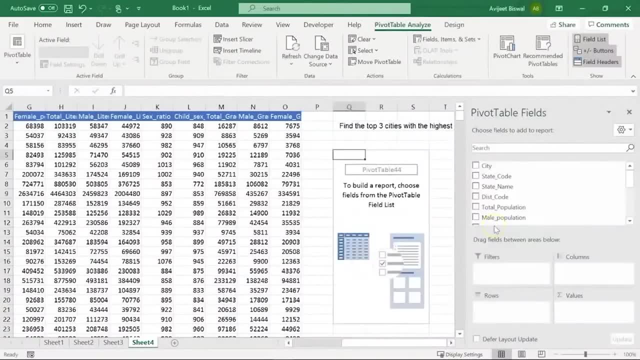 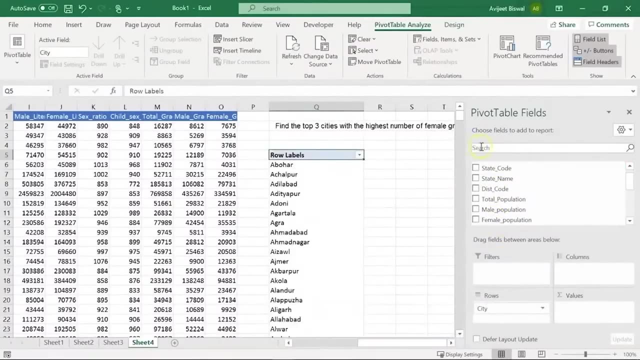 click on the pivot table option, go to existing worksheet, click on q5 and hit ok. now, since we want to find the top three cities, i'll drag the city column onto rows. and then we want the female graduates. so in the search bar i'll look for. 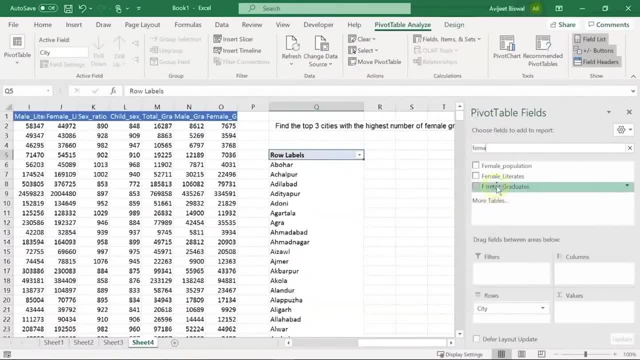 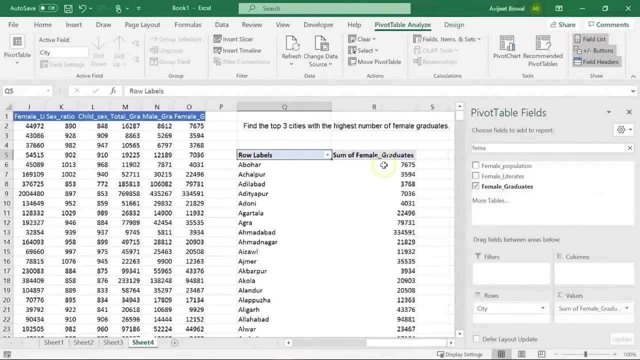 female, and i'll choose this column, that is, female graduates, and drag it here onto values. so i have the sum of female graduates for each of the cities now, since we want to find the highest number of female graduates in the top three cities. so let me first sort this column. 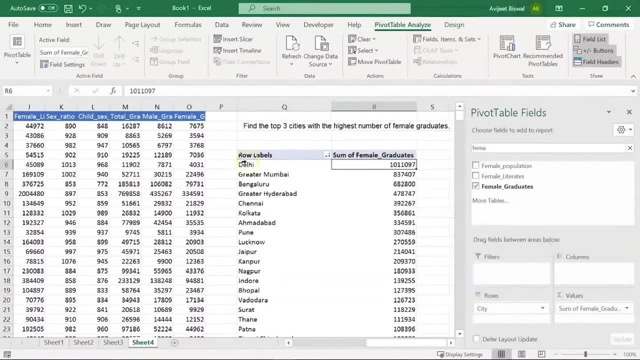 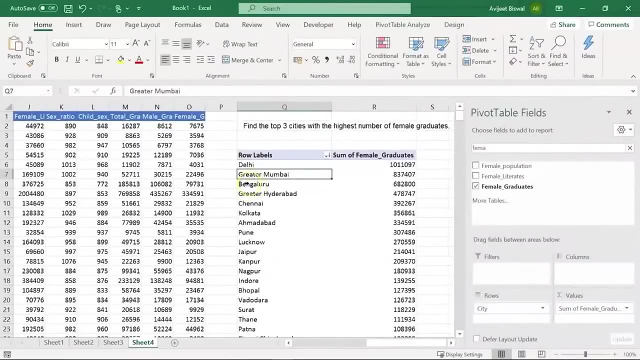 i'll sort it in descending order. now we have it sorted now. from this you can see that delhi, greater mumbai and bangalore are the top three cities, but it's displaying all the cities for us, so let's filter only the top three. so what you can do is right. 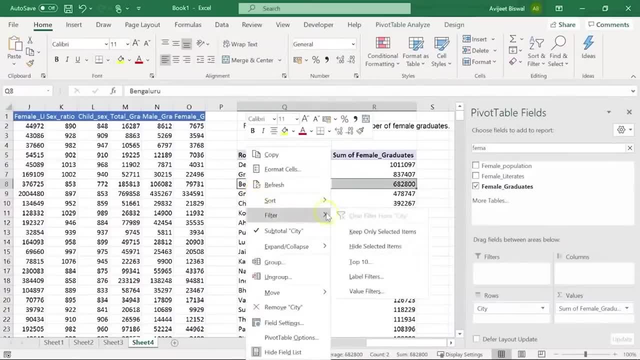 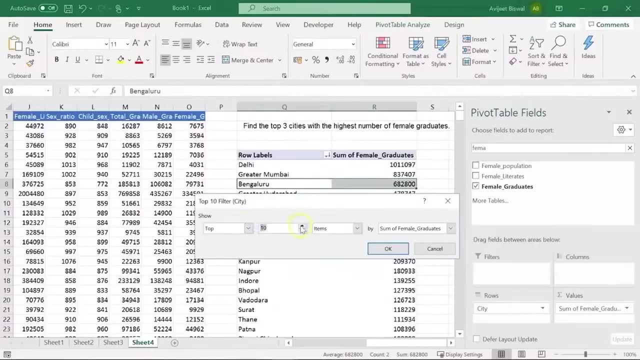 click and go to filter. under filter you have the option of top 10. i'll select this here. i only want the top three, so either you can go down like this or you can directly type 3. your column is already selected. let me just click on. ok. 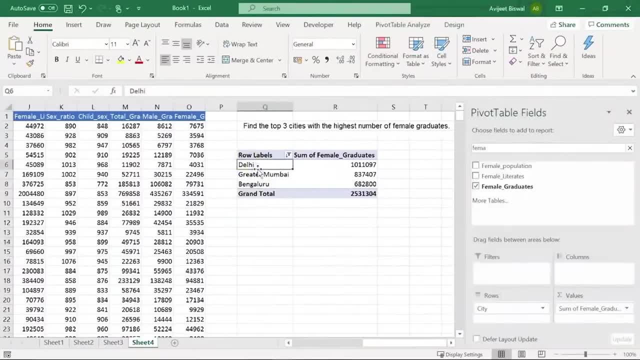 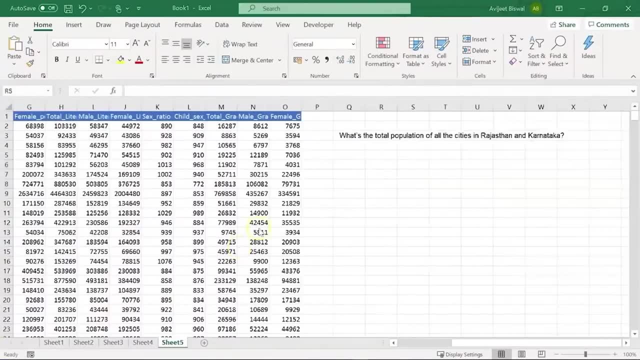 there you go. we have the required pivot table ready, and it only displays us the top three cities with the highest number of female graduates. now the next thing we want to see is how to use a slicer in a pivot table. so we have a question here. what's the 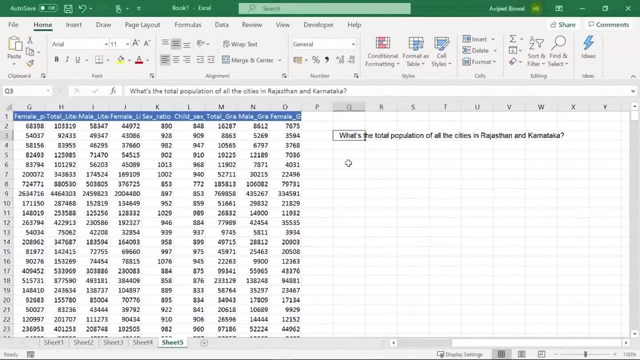 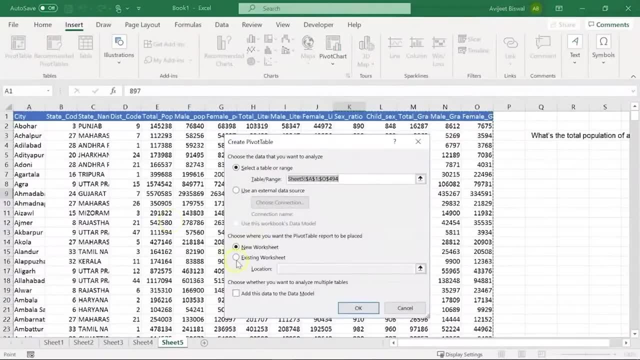 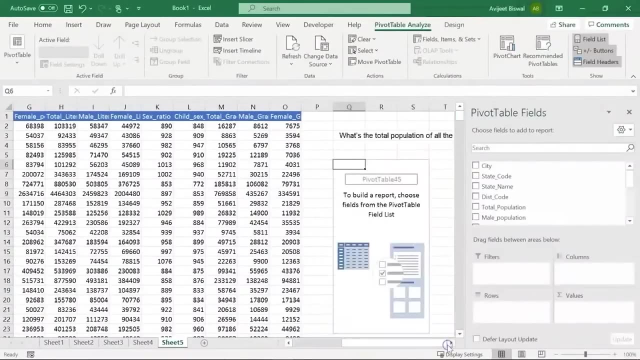 total population for all the cities in rajasthan and karnataka. so let's create a pivot table for this and see how you can use a slicer to filter the table. click on existing. i'll click on a location this time: q6. click ok now, since i want the total population. 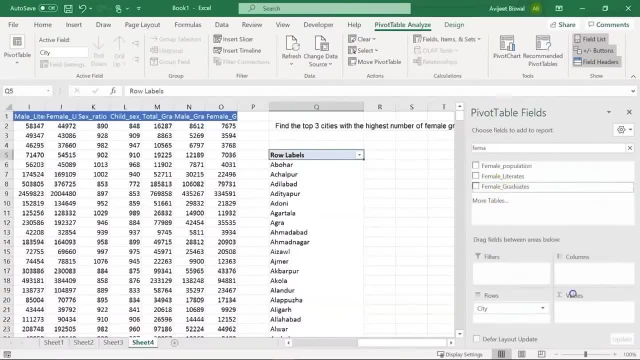 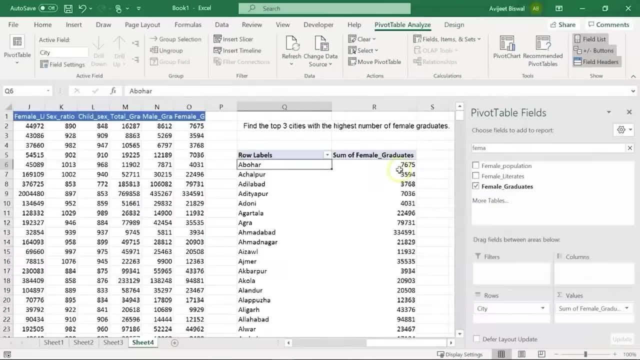 and i'll choose this column, that is, female graduates, and drag it here onto values. so i have the sum of female graduates for each of the cities now, since we want to find the highest number of female graduates in the top three cities. so let me first sort this column. 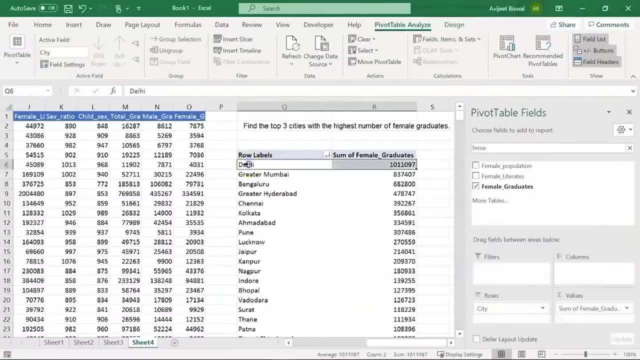 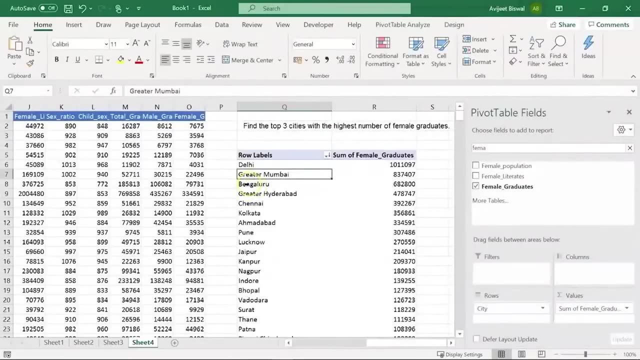 i'll sort it in descending order. now we have it sorted. now. from this you can say that delhi, greater mumbai and bangalore are the top three cities, but it's displaying all the cities for us, so let's filter only the top three. so what you can. 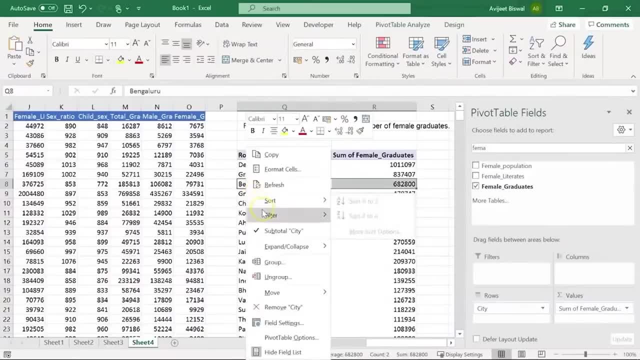 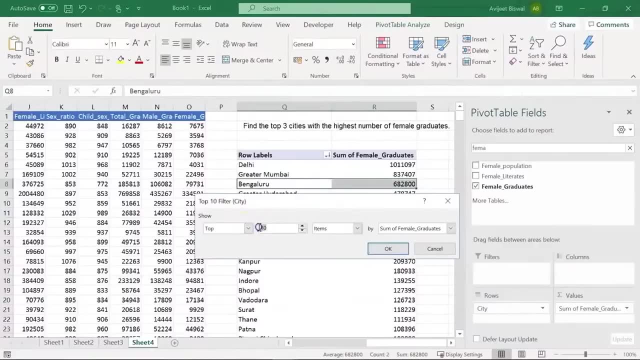 do is right click and go to filter. under filter you have the option of top ten. i'll select this here. i only want the top three, so either you can go down like this or you can directly type three. your column is already selected. let me just click on. ok. 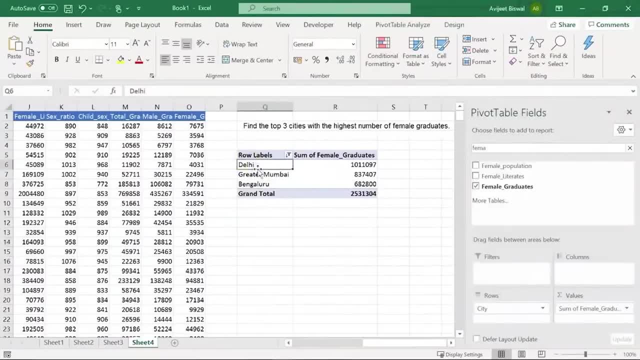 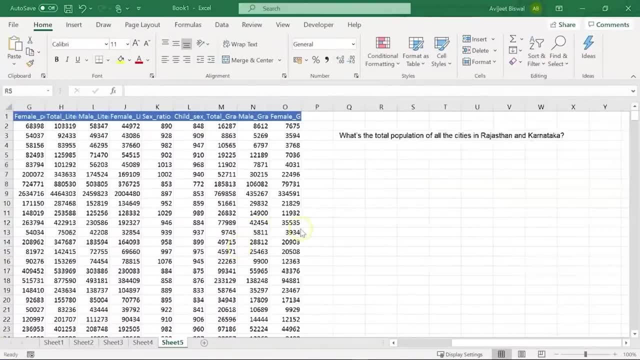 there you go. we have the required pivot table ready, and it only displays us the top three cities with the highest number of female graduates. now the next thing we want to see is how to use a slicer in a pivot table. so we have a question here. what's the total? 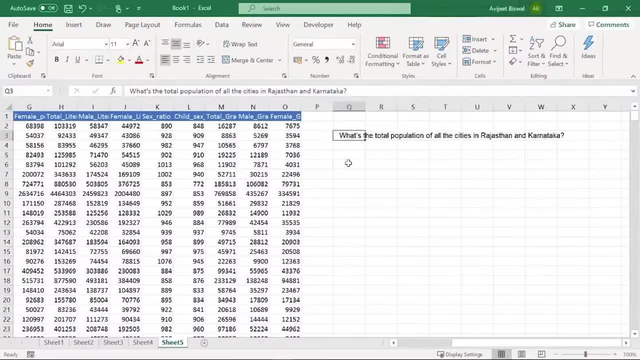 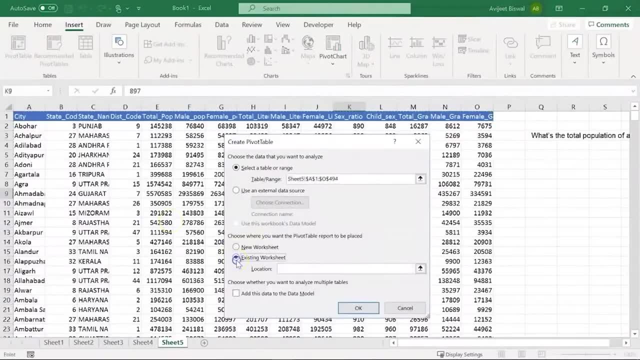 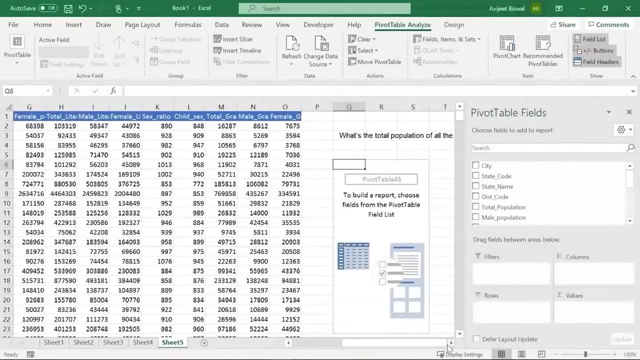 population for all the cities in rajasthan and karnataka. so let's create a pivot table for this and see how you can use a slicer to filter the table. click on existing. i'll click on a location this time: q6. click ok now, since i want the total population. 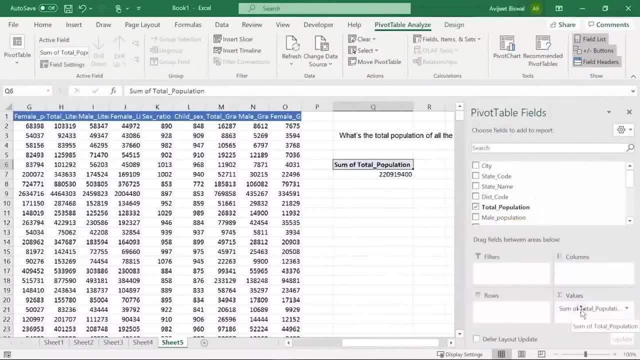 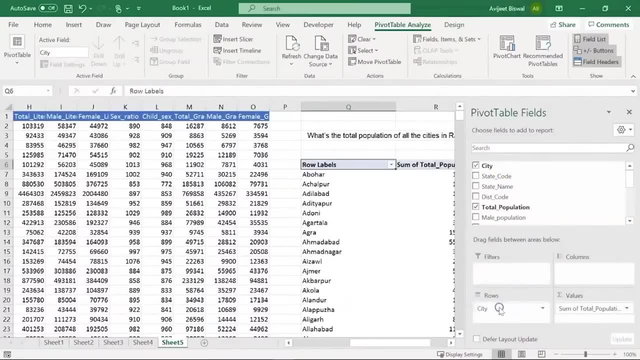 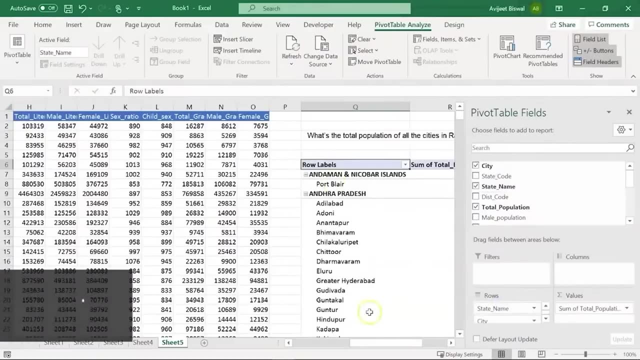 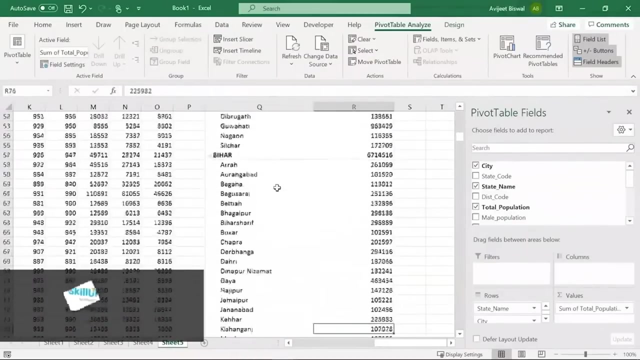 so i'll drag total population onto values and then i'll select the city onto rows and then the state name. also i'll place it on top of city. so you have in the pivot table all the states and their cities and on the right you can see the total population for each of these. 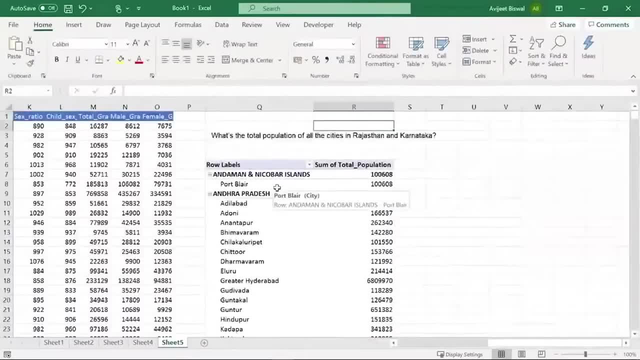 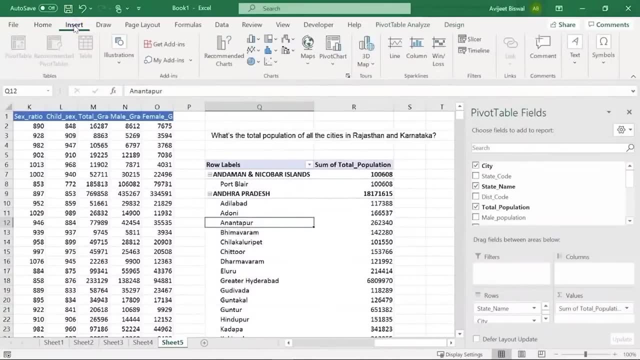 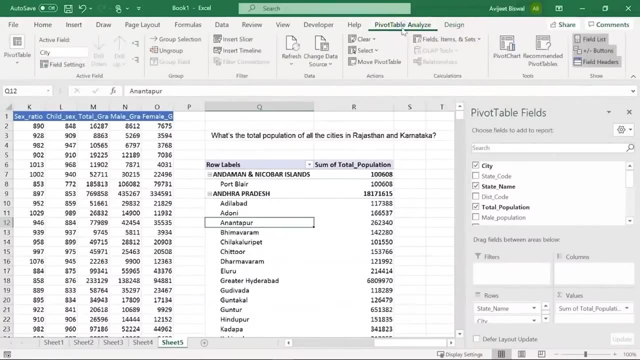 cities. but our question is: we want to find only for rajasthan and karnataka now. for that, what you can do is go to insert and create a slicer. either you can create from this option or you can go to pivot table analyze option and here you have the option to create. 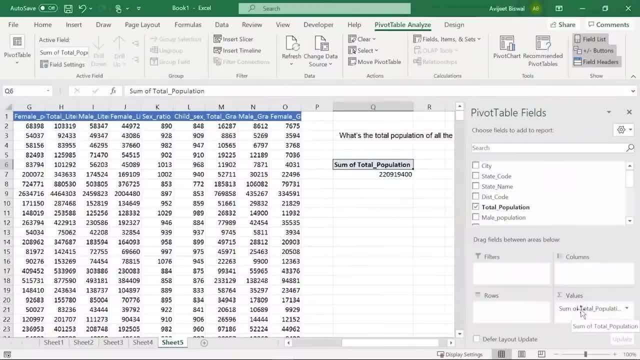 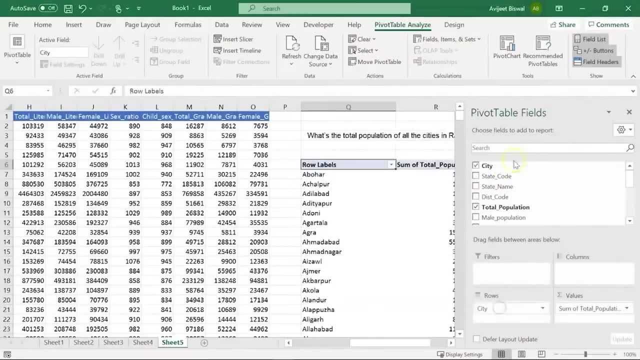 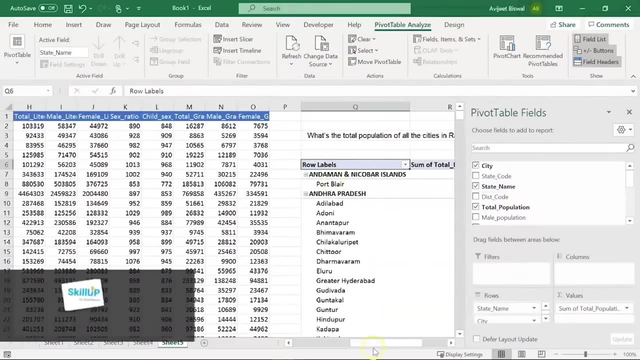 so i'll drag total population onto values and then i'll select the city onto rows and then the state name. also i'll place it on top of city. so you have in the pivot table all the states and their cities and on the right you can see: 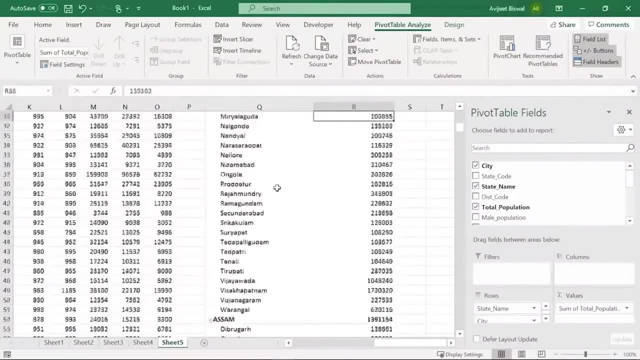 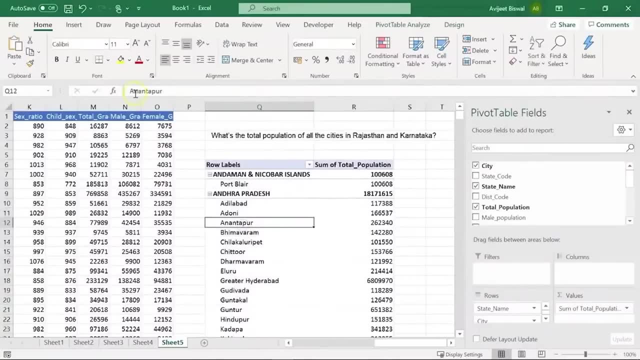 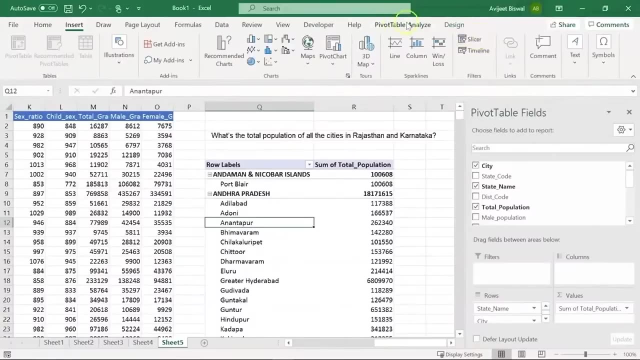 the total population for each of these cities. but our question is: we want to find only for rajasthan and karnataka. now for that, what you can do is go to insert and create a slicer. either you can create from this option or you can go to. 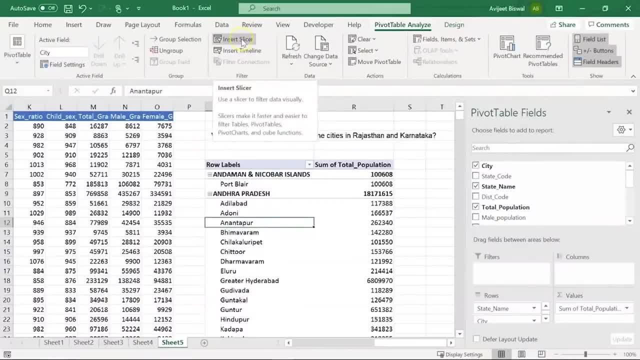 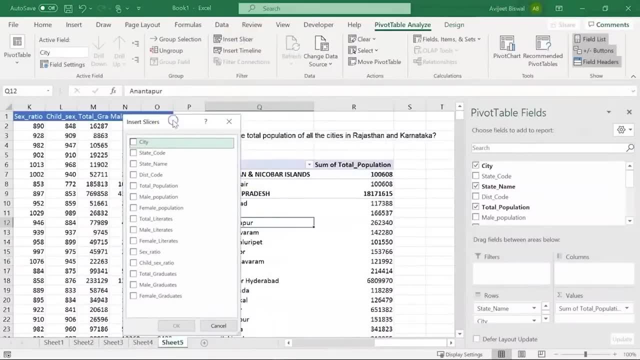 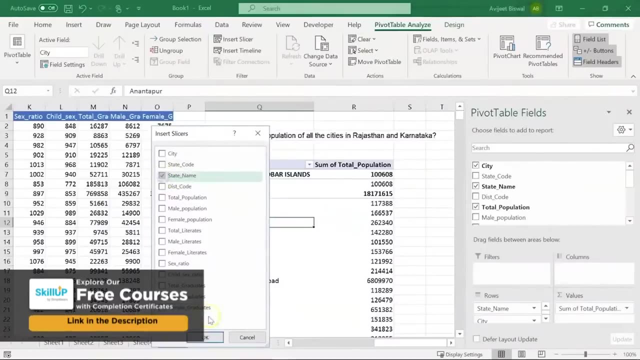 pivot table analyze option and here you have the option to create or insert a slicer and click on this and since we want to slice the table based on state- that is, rajasthan and karnataka- i'll choose state name as my slicer field. you can see: 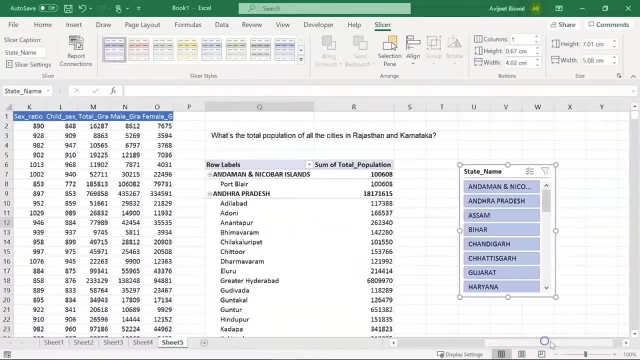 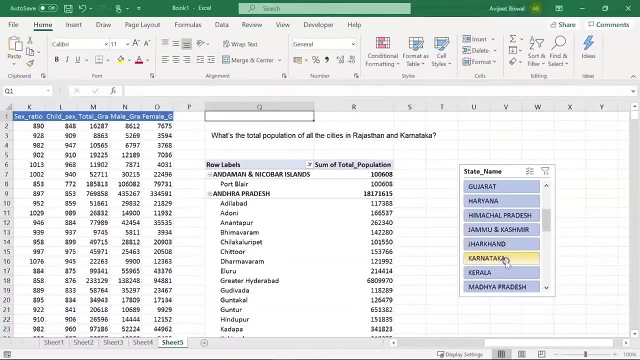 this is my slicer here. now you only want the data for rajasthan and karnataka, so i'll search for these two. so here we have karnataka, so let me select karnataka first. and i also want for rajasthan, so let me select. 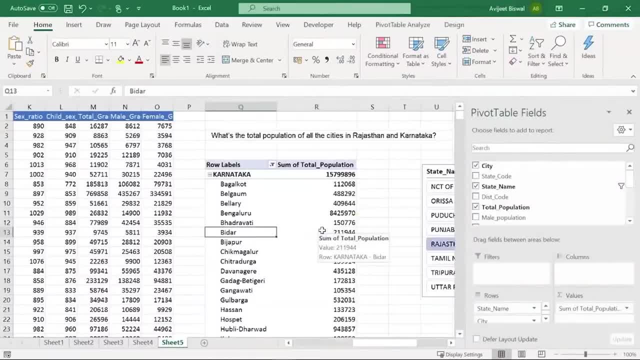 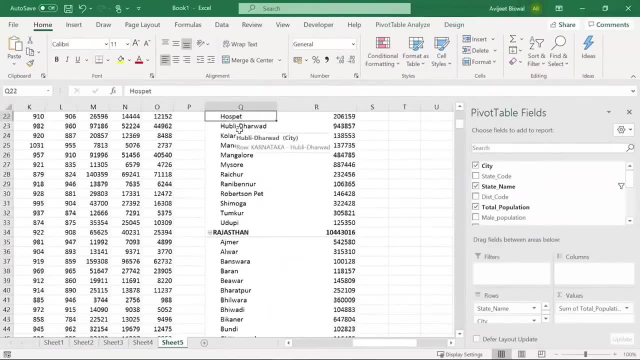 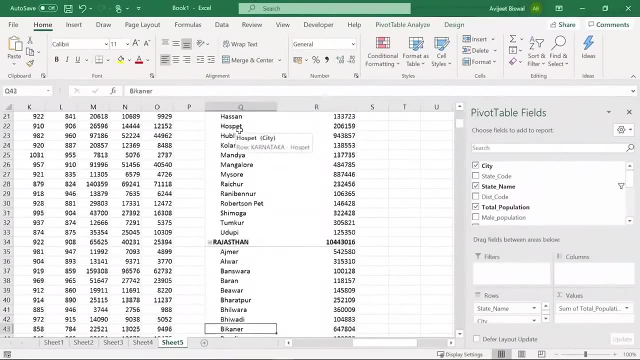 rajasthan also. you can see in our pivot table we only have data for rajasthan and karnataka. so this pivot table shows you different cities from karnataka and the total sum of population from each of the cities, and similarly we also have for rajasthan. 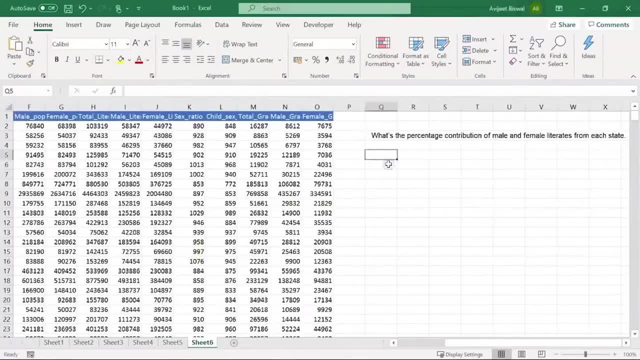 moving ahead now we will see another very interesting feature of pivot, that is, you can create percentage contribution of a table, for example. we have a question here: what's the percentage contribution of male and female literates from each state? now we want to see in terms of. 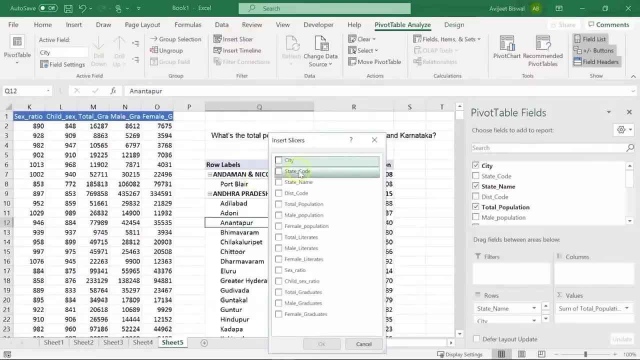 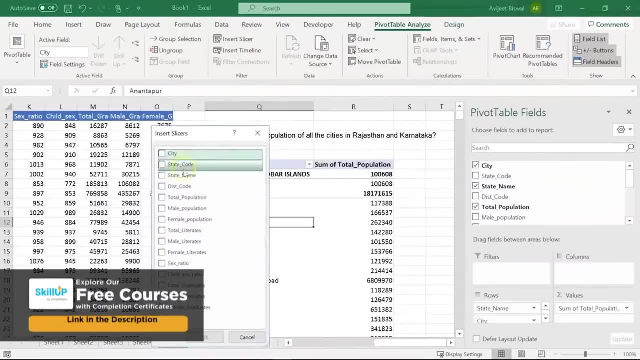 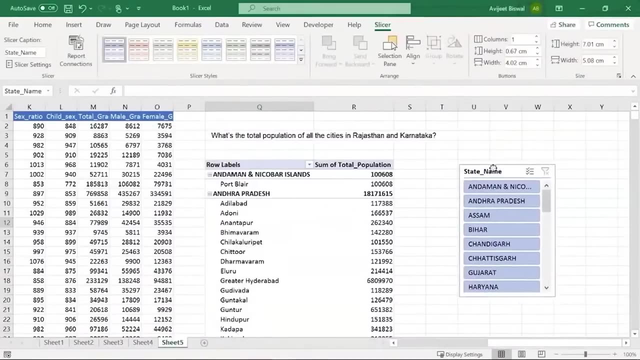 or insert a slicer. i'll click on this and since we want to slice the table based on state- that is, rajasthan and karnataka- i'll choose state name as my slicer field. you can see, this is my slicer here now you only want. 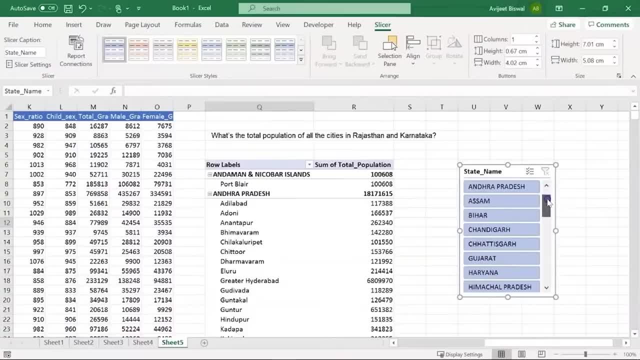 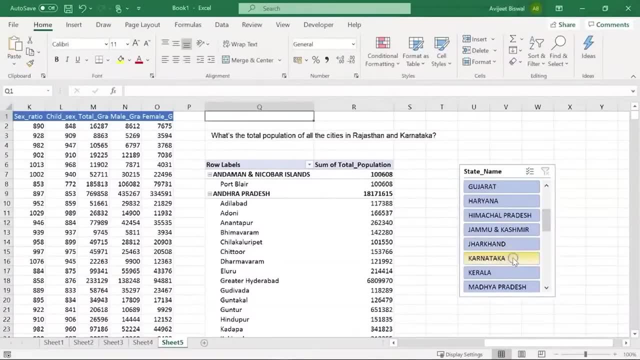 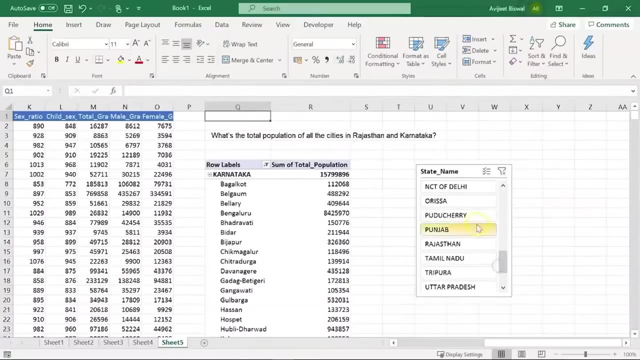 the data for rajasthan and karnataka, so i'll search for these two. so here we have karnataka, so let me select karnataka first. and i also want for rajasthan, so let me select rajasthan also. you can see, in our pivot table we only have 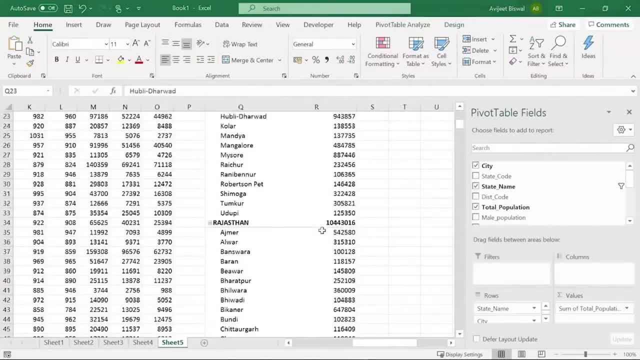 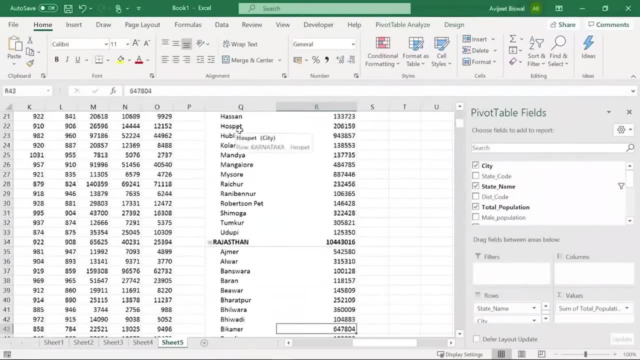 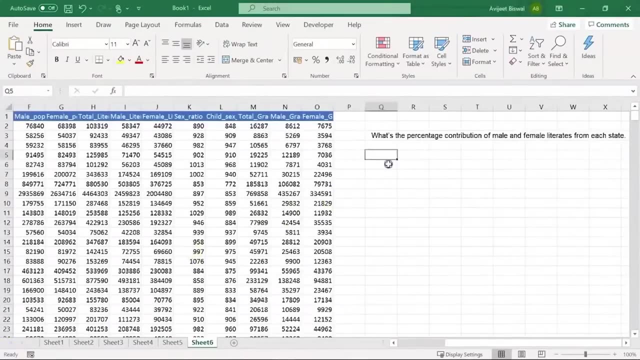 data for rajasthan and karnataka. so this pivot table shows you different cities from karnataka and the total sum of population from each of the cities, and similarly we also have for rajasthan. moving ahead now we will see another very interesting feature of pivot, that is: 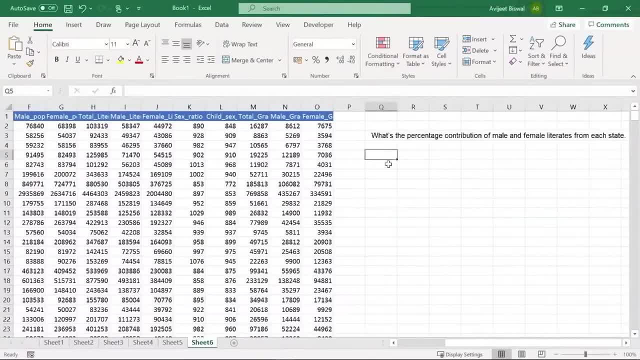 how you can create percentage contribution of a table. for example, we have a question here: what's the percentage contribution of male and female literates from each state? now, we want to see in terms of percentage and not as sum or average. so let's do that. i'll create my pivot table. 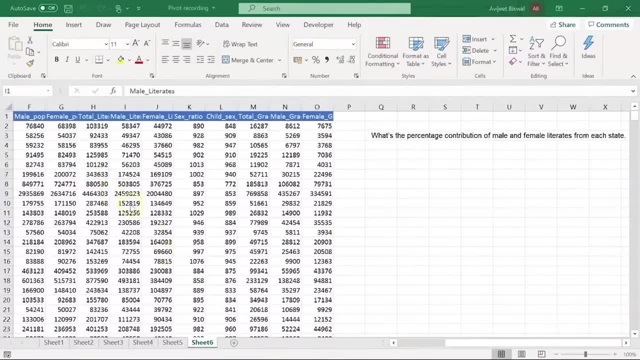 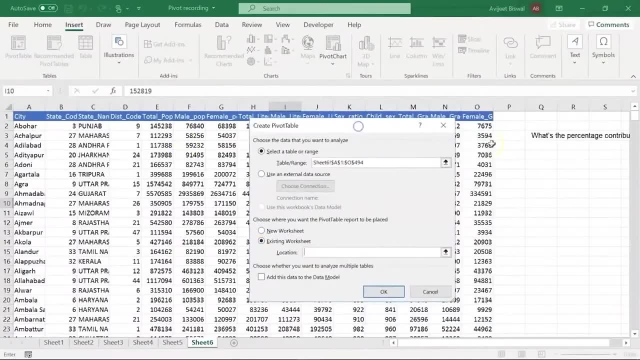 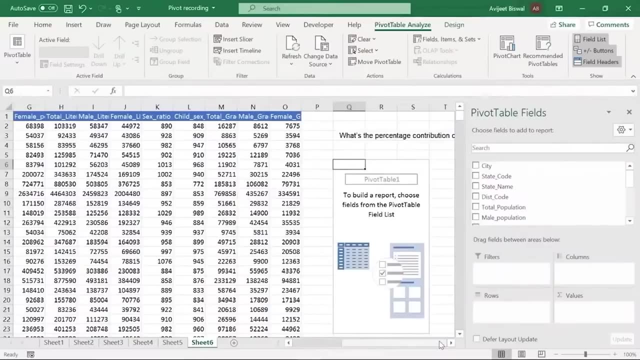 percentage and not as sum or average. let's do that. i'll create my pivot table, click on existing and i'll select an empty cell. okay, now here, since we want to find the percentage contribution of male and female literates, so first i'll drag male literates. 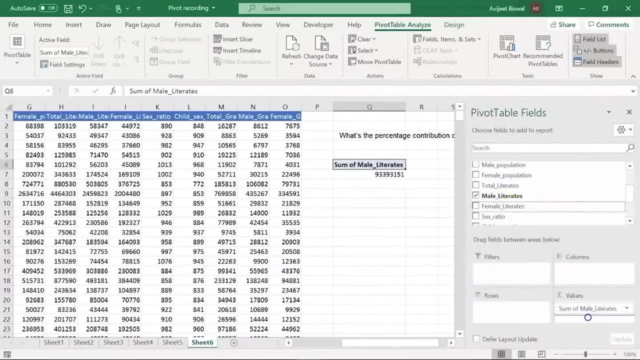 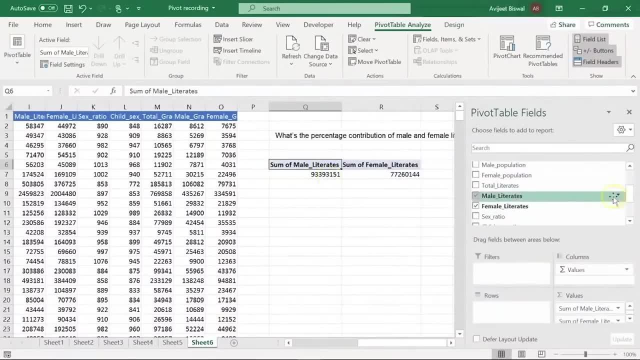 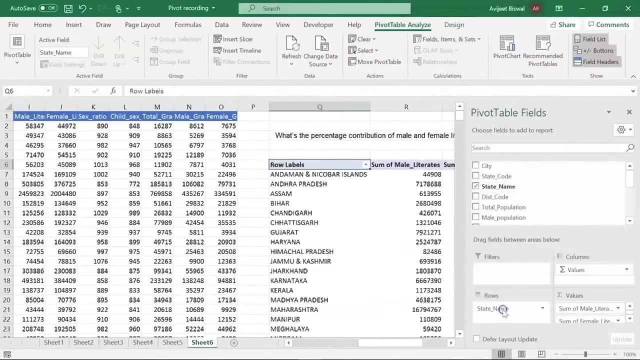 onto values, followed by female literates onto values. by default it has summed up the male literates and female literates value and also i want to drag state column to rows. so here you can see the sum of male literates and female literates per state i want to convert. 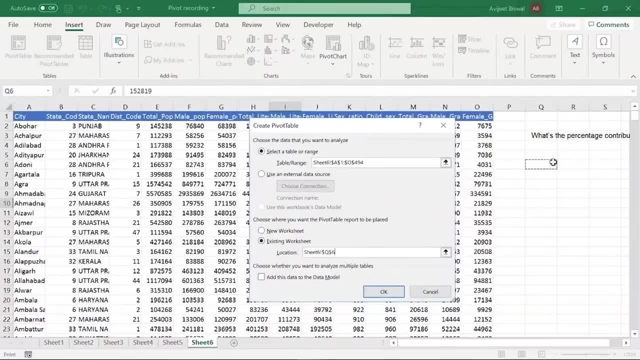 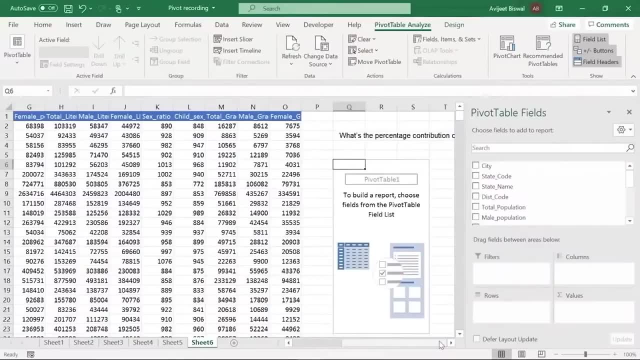 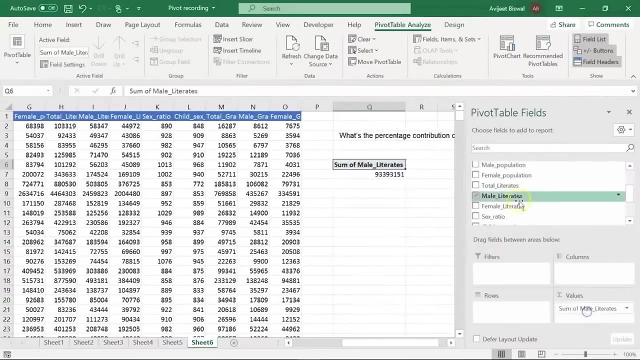 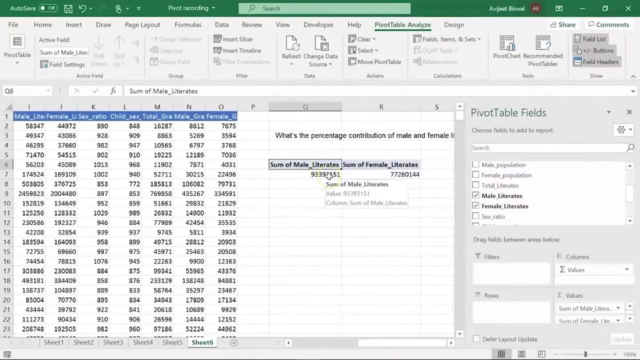 click on existing and i'll select an empty cell. ok, now here, since we want to find the percentage contribution of male and female literates. so first i'll drag male literates onto values, followed by female literates onto values. by default, it has summed up the male literates and female literates. 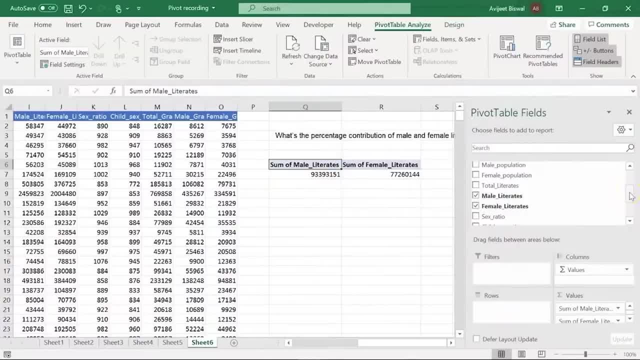 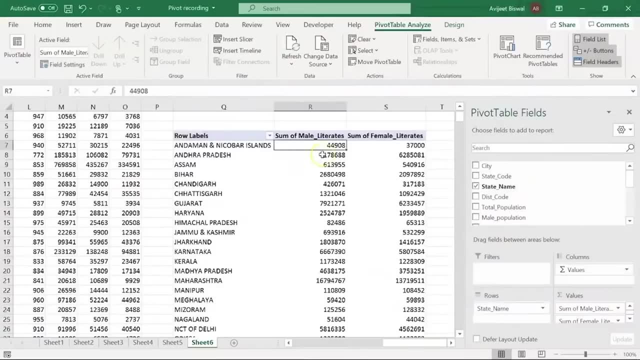 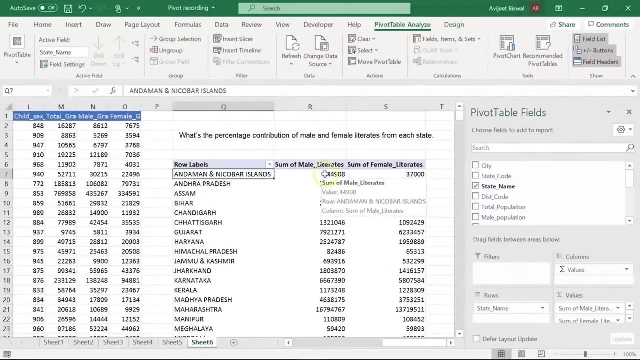 value, and also i want to drag state column to rows. so here you can see the sum of male literates and female literates per state. i want to convert this as percentage contribution. so what we can do is i'll select any cell and i'll right click. 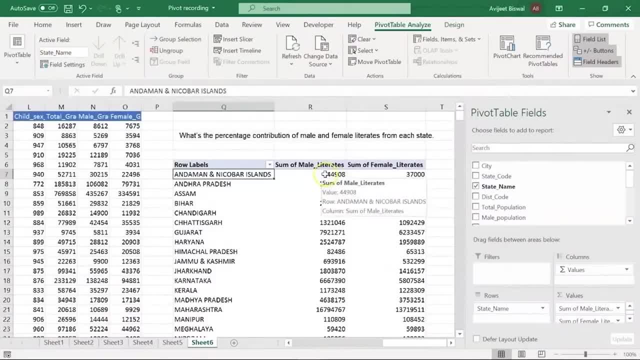 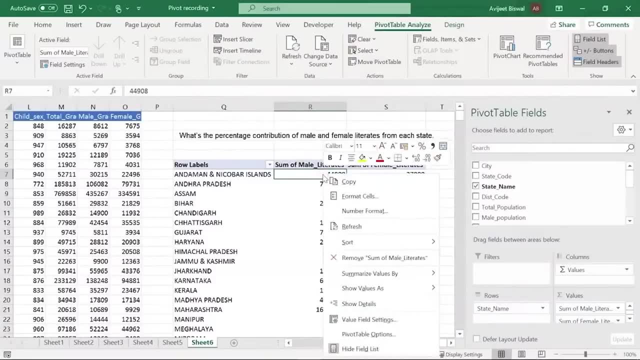 this as percentage contribution. so what we can do is i'll select any cell and i'll right click and i'll go to so value as- and here i have the option to select percentage of grand total. so i'll select this. you can see we have the percentage contribution of. 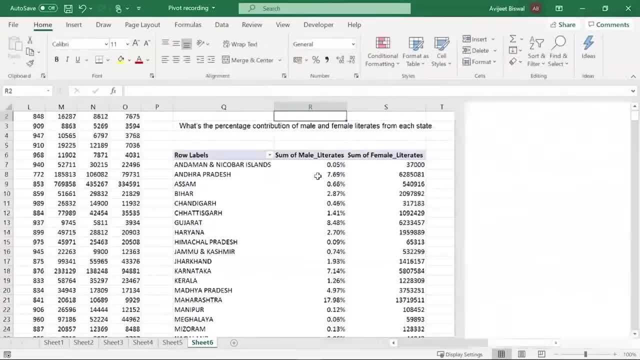 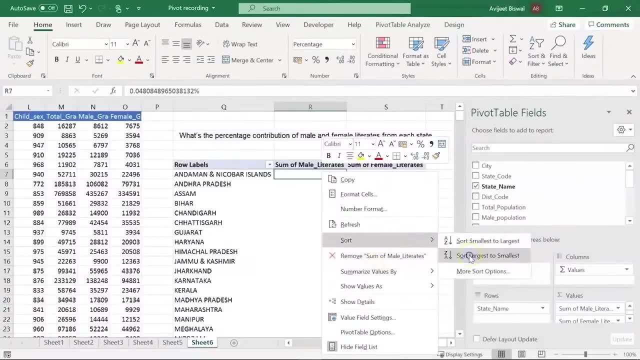 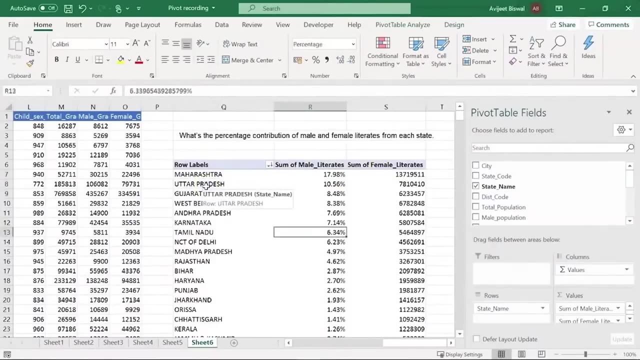 male literates to the total. now, if i sort this, you will get to know which state contributed or has the highest percentage contribution. so we have Maharashtra for male literates. then we had Uttar Pradesh. in 2011, if i come down, we had Meghalaya. 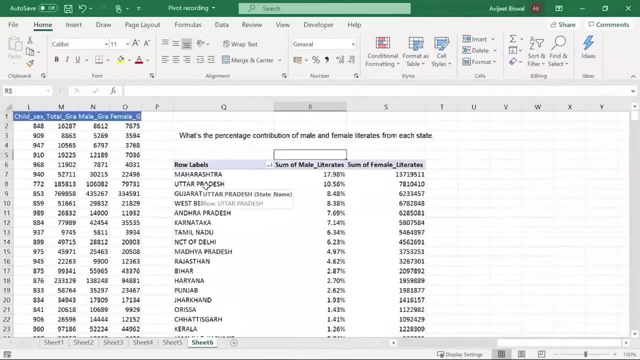 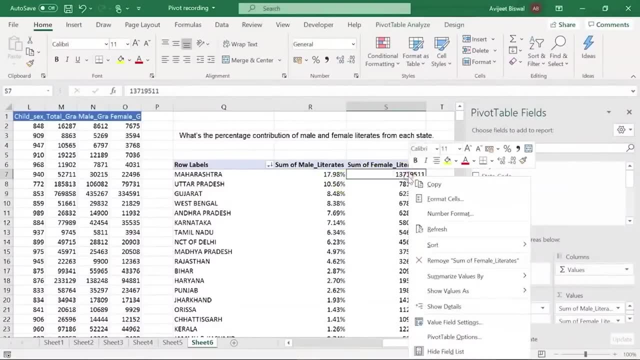 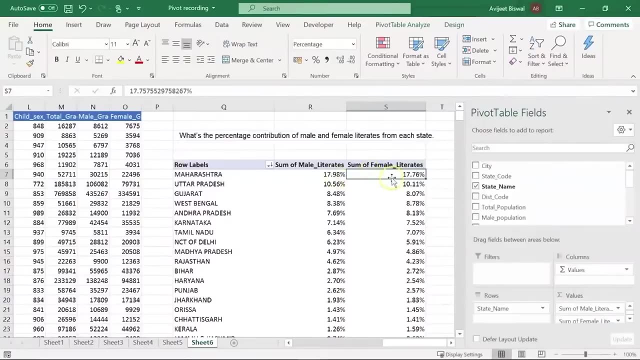 Nagaland and Andaman and Nicobar islands as those states which had little or minimal contribution to male literates. similarly, let's do it for female literates. i'll go to so value as and select percentage of grand total so you can see here also Maharashtra, Uttar Pradesh. 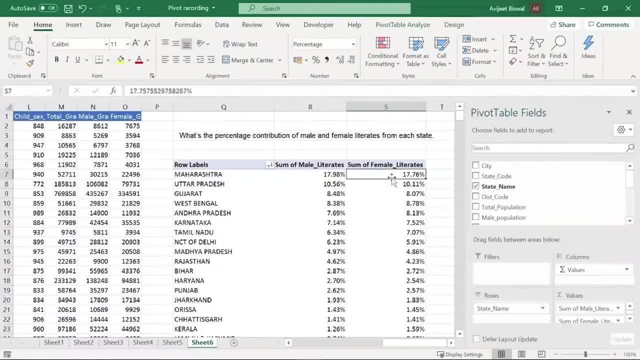 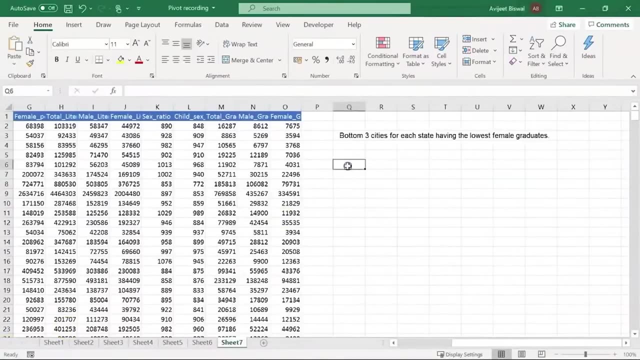 then Gujarat, and all had the highest percentage contribution to female literates. so this is another good feature: to convert your data and see it in terms of percentage. now moving ahead, let's say we want to find the bottom three cities from each state that had the lowest female 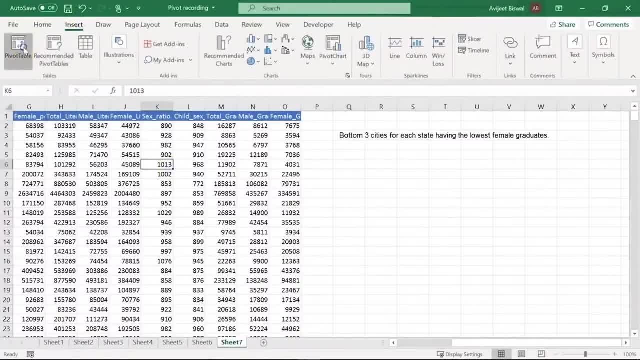 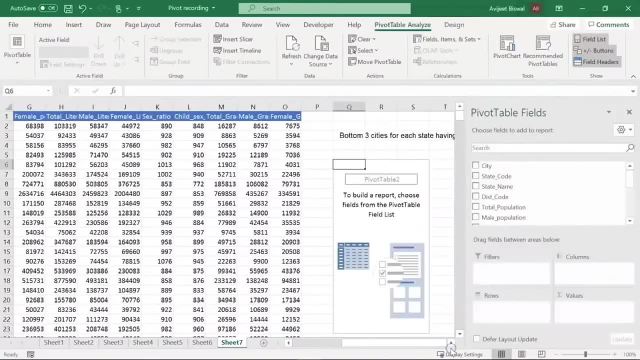 graduates. we can do that as well. i'll go to insert, click on pivot, go to existing worksheet, select an empty worksheet and click on ok now, since i want to see based on states as well as cities, so let me drag the state name first onto rows and let's drag 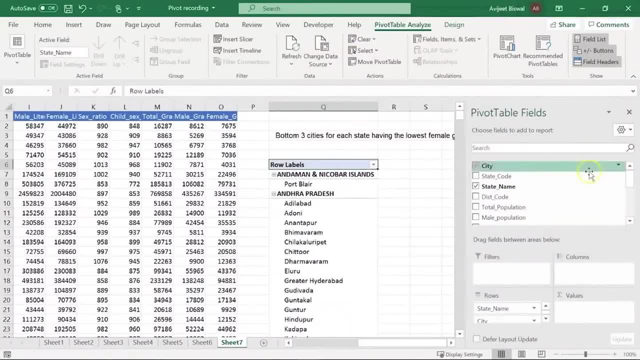 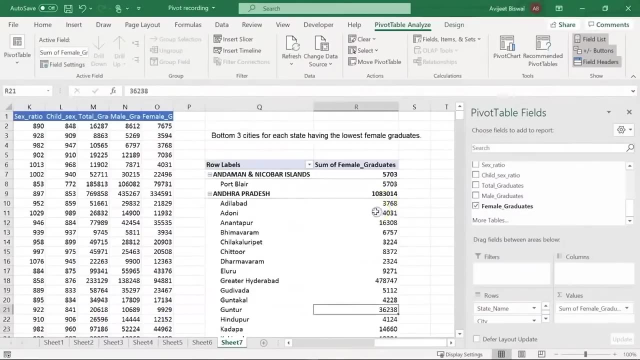 city column onto rows. next, we want female graduates, so let me look for female graduates in the field list. i'll drag it onto values. now we have the list of states and their respective cities, and to the right of the pivot table you can see the sum of female. 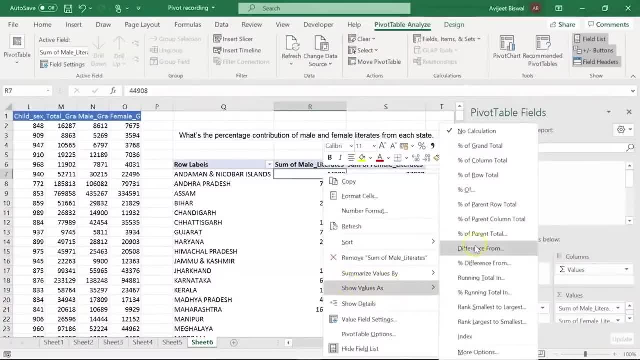 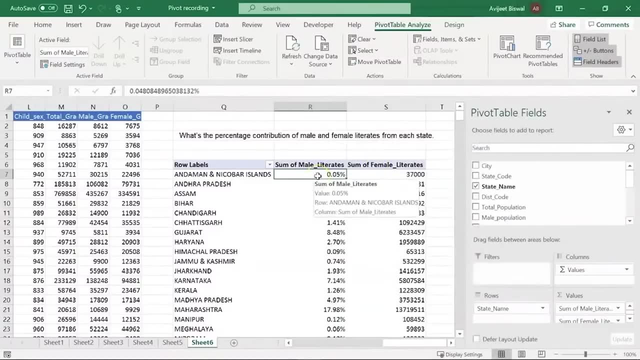 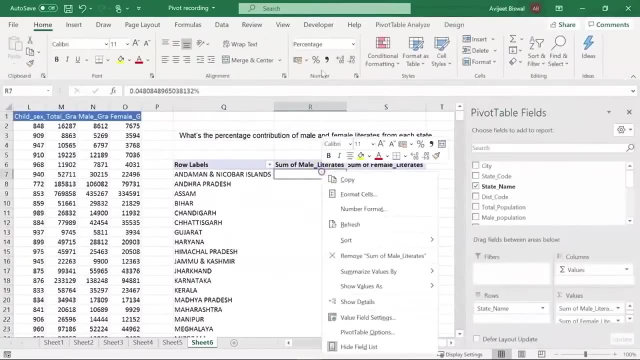 and i'll go to so value as and here i have the option to select percentage of grand total, so i'll select this. you can see we have the percentage contribution of male literates to the total. now, if i sort this, you will get to know which. 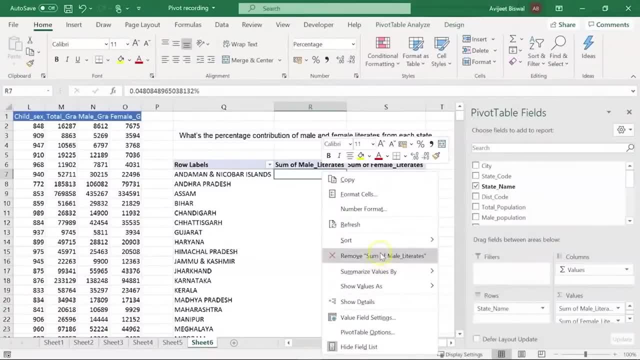 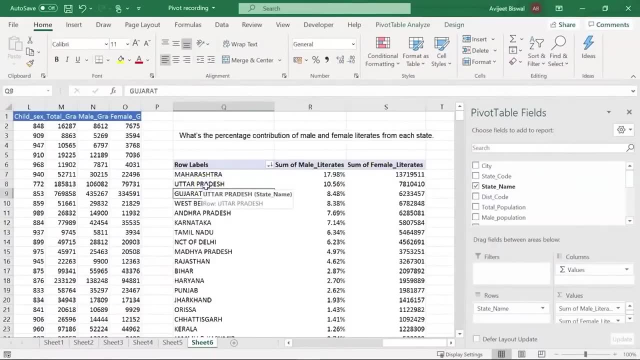 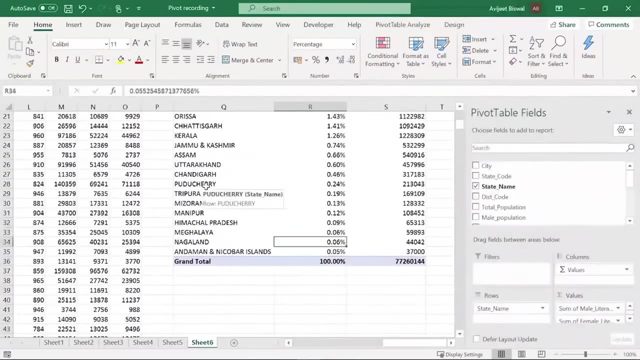 state contributed or has the highest percentage contribution. so we have maharashtra for male literates. then we had uttar pradesh. in 2011, if i come down, we had mighalaya, nagaland and andaman and nicobar islands as those states which had little or 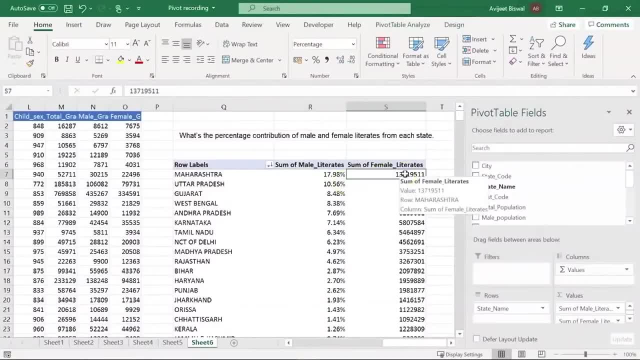 minimal contribution to male literates. similarly, let's do it for female literates. i'll go to so value as and select percentage of grand total. so you can see here also maharashtra, uttar pradesh, then gujarat, and all had the highest percentage contribution to female. 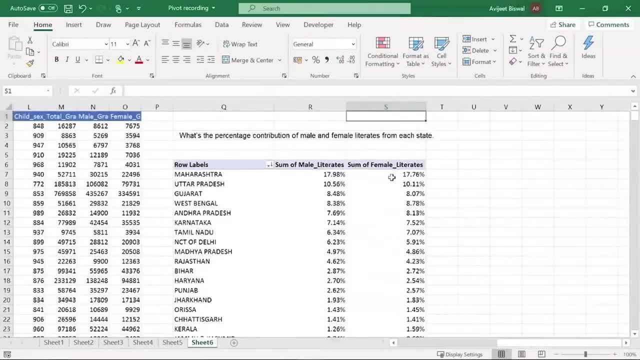 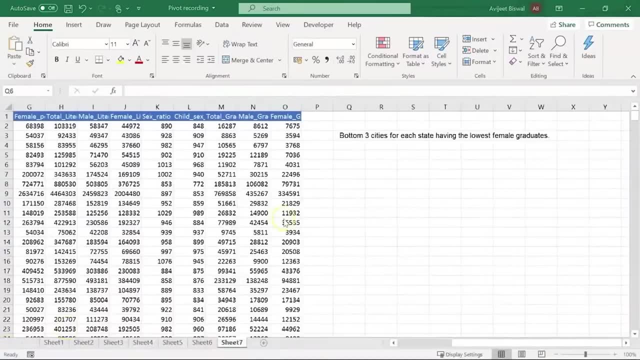 literates. so this is another good feature: to convert your data and see it in terms of percentage. now moving ahead, let's say we want to find the bottom three cities from each state that had the lowest female graduates. we can do that as well. i'll go to. 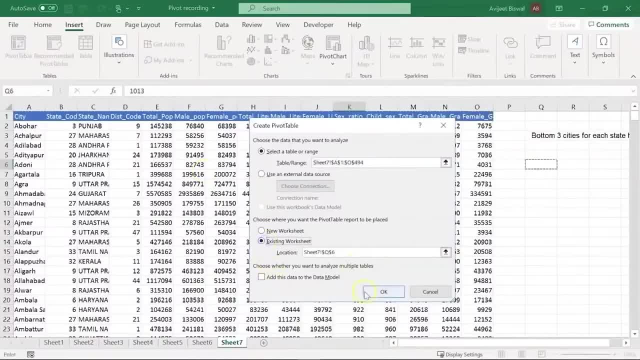 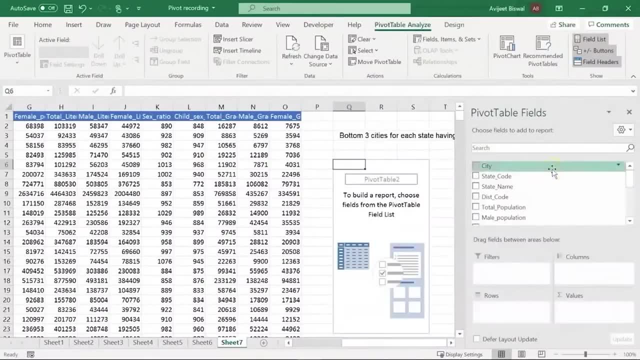 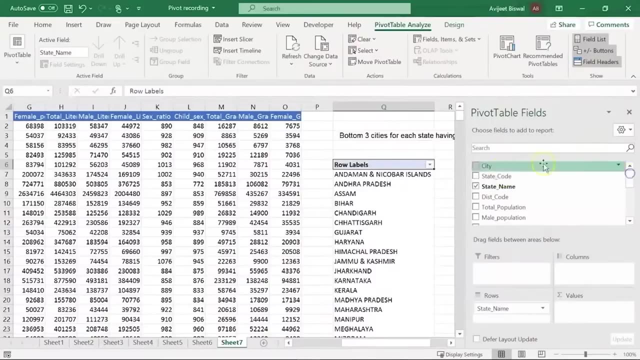 insert, click on pivot, go to existing worksheet, select an empty worksheet and click on ok now, since i want to see based on states as well as cities, so let me drag the state name first onto rows and let's drag the city column onto rows next. we want female graduates. 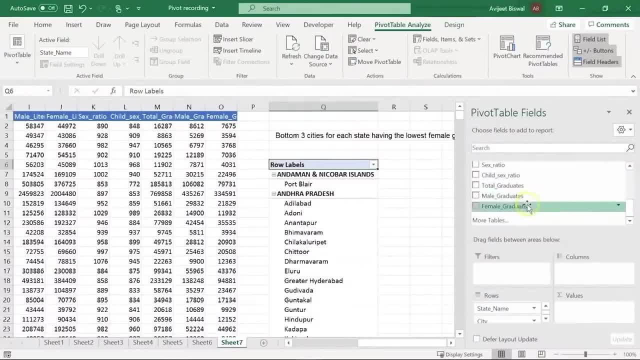 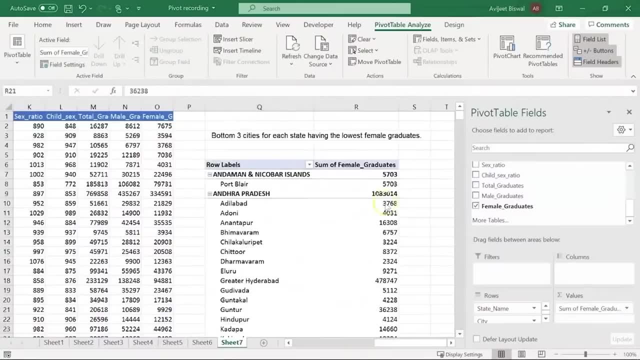 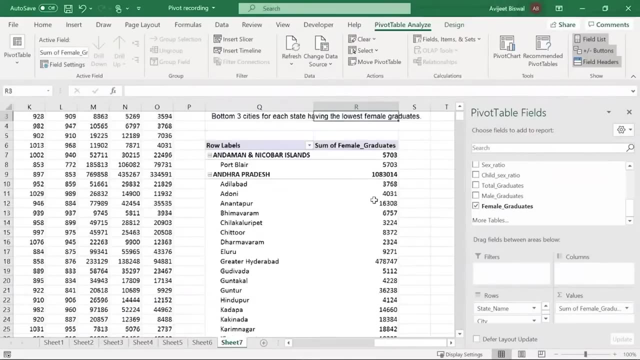 so let me look for female graduates in the field list. i'll drag it onto values. now we have the list of states and their respective cities, and to the right of the pivot table you can see the sum of female graduates from each city. now, first i will sort this column. 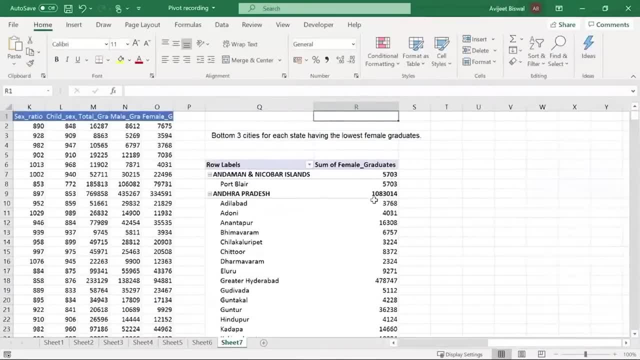 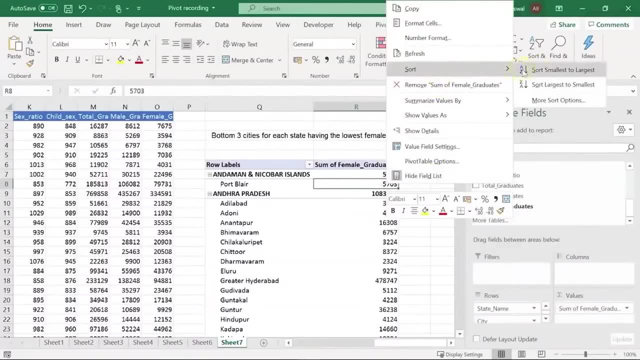 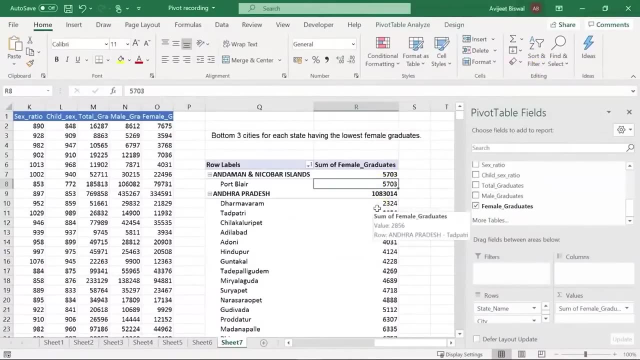 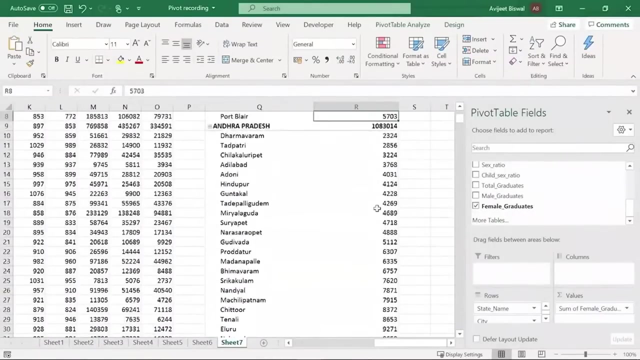 graduates from each city. now first i'll sort this column. i'll right click, go to sort and click on shortest to largest. now we have sorted our female graduates from shortest or smallest to largest. now, since i want to find the bottom three cities from each state, i'll come to this cell. 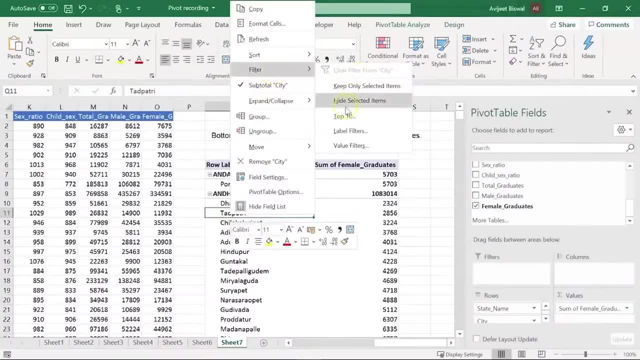 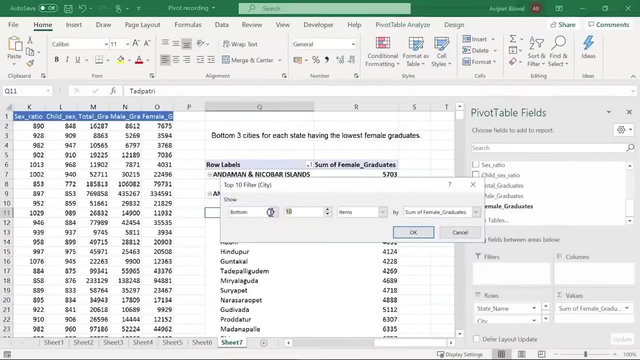 right click, go to filter and select top 10. now i'll replace top 10 with bottom and i want the bottom three cities from each state. i have my column selected. that is sum of female graduates. if i click on ok, you can see here some of the states. don't have three cities. so you can see andaman and ukber islands has only one city that is port player, while the remaining you can find the bottom three cities with the lowest number of female graduates. so andhra pradesh had these three in assam. 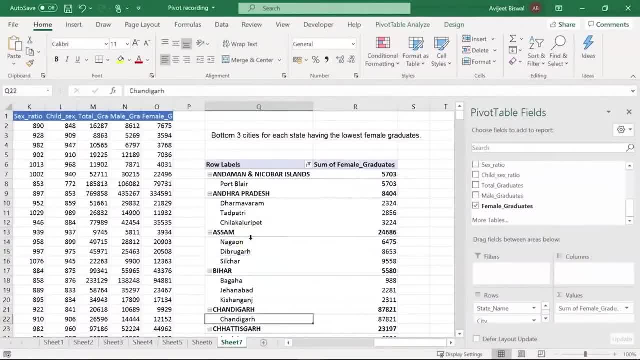 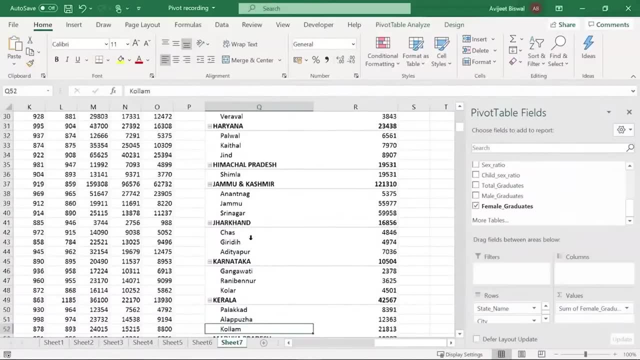 we had nagaon, then there was tiburgarh and selcha. similarly, if i come down in haryana we have palwal, kathal and zind. if i come further here you can see. for karnataka there is gangavati. 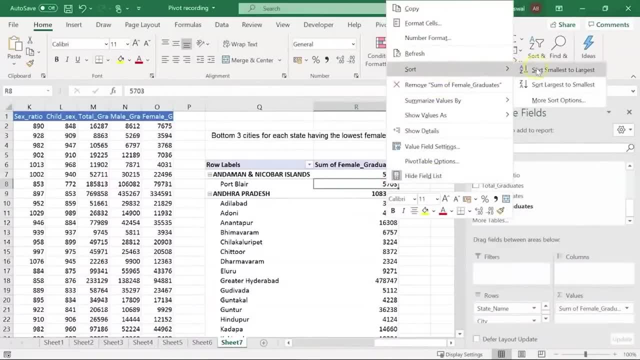 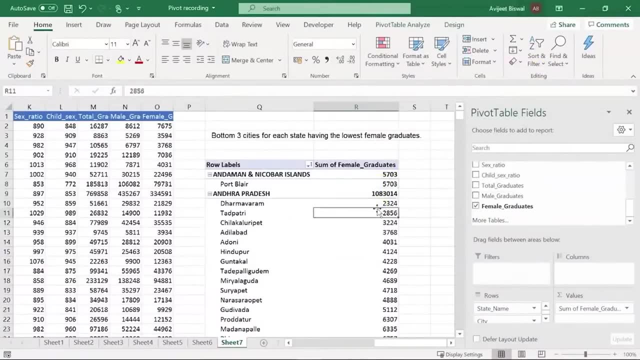 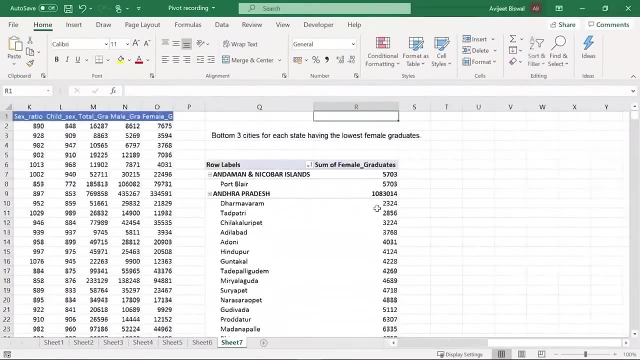 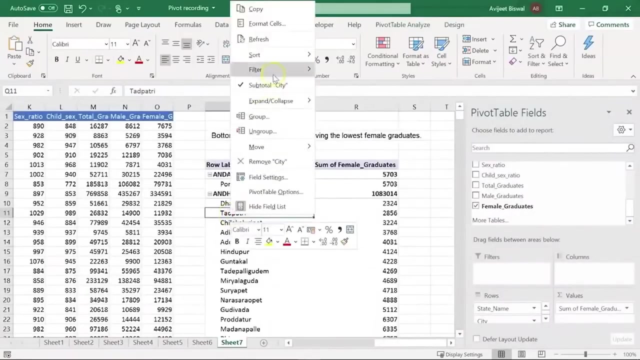 i'll right click, go to sort and click on shortest to largest. now we have sorted our female graduates from shortest or smallest to largest. now, since i want to find the bottom three cities from each state, i'll come to the cell, right click, go to filter and select top 10. 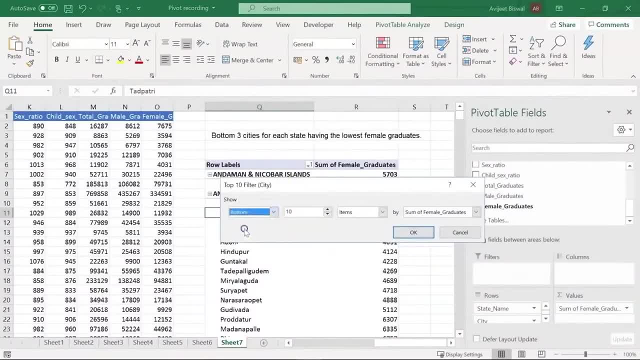 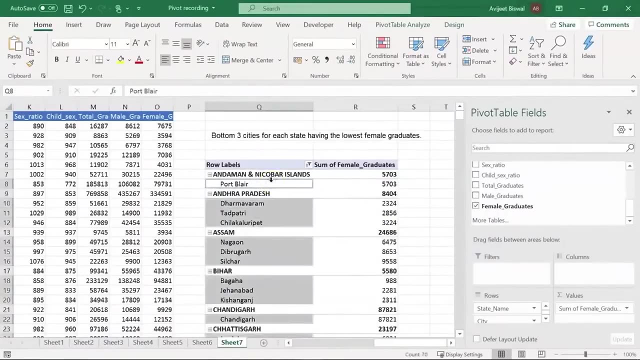 now i'll replace top 10 with bottom and i want the bottom three cities from each state. i have my column selected. that is sum of female graduates. if i click on ok, you can see here. some of the states don't have three cities, so you can see Andaman and Nicobar islands. 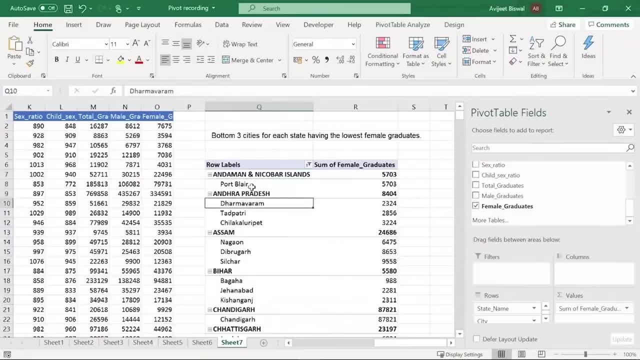 has only one city, that is, Port Blair, while the remaining you can find the bottom three cities with the lowest number of female graduates. so Andhra Pradesh had these three. in Assam, we had Nagaon, then there was Dibrugarh and Silchar. similarly, if i come, 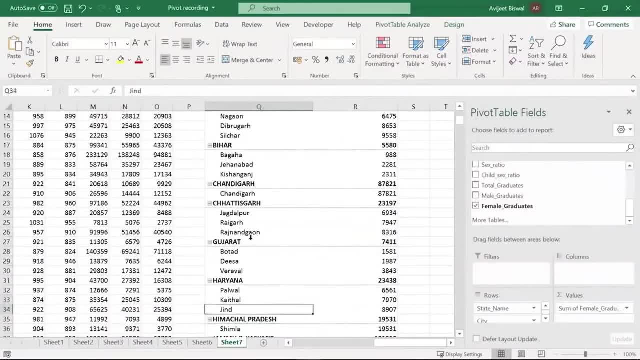 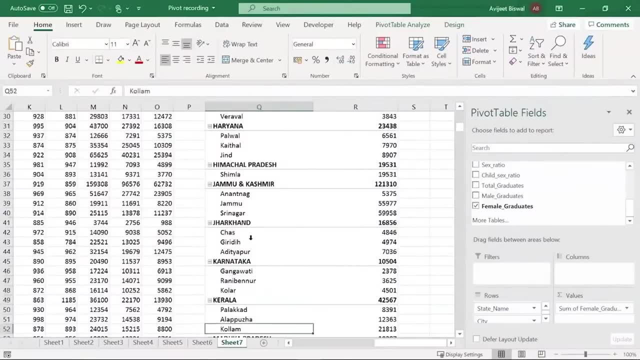 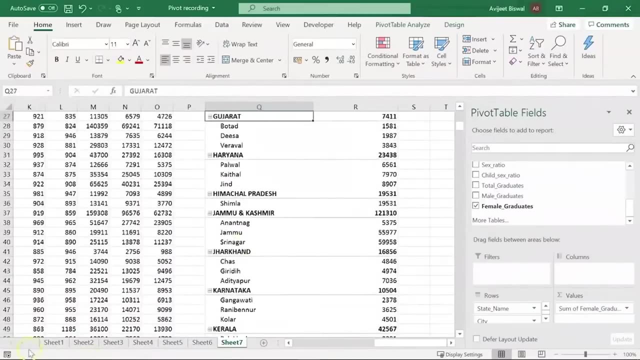 down in Haryana, we have Palwal, Kathal and Zind. if i come further here, you can see for Karnataka: there is Gangavati, there is Rani Benur and there is Kolar. similarly you can see for Kerala as well. now, moving ahead, now in the next example, 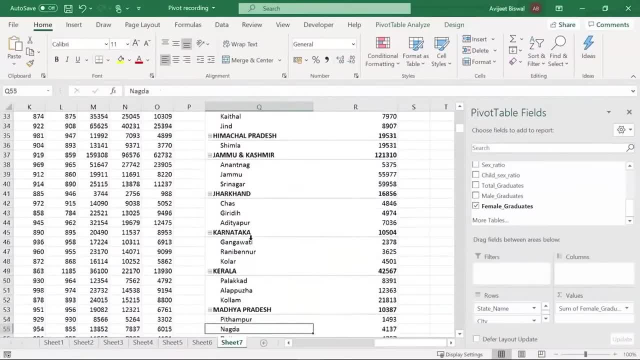 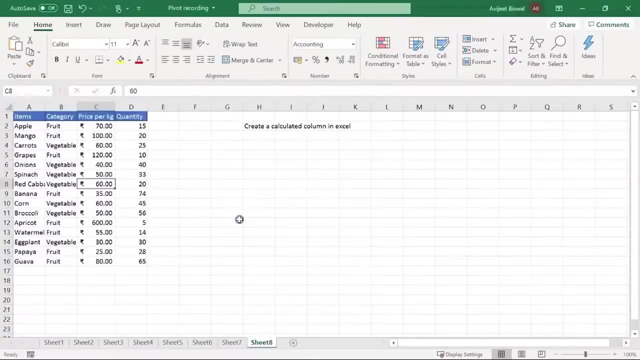 there is ranibanur and there is kolar. similarly you can see for kerala as well. now, moving ahead now, in the next example, i'll tell you how you can create a calculated field or a calculated column in excel with the help of a pivot table. 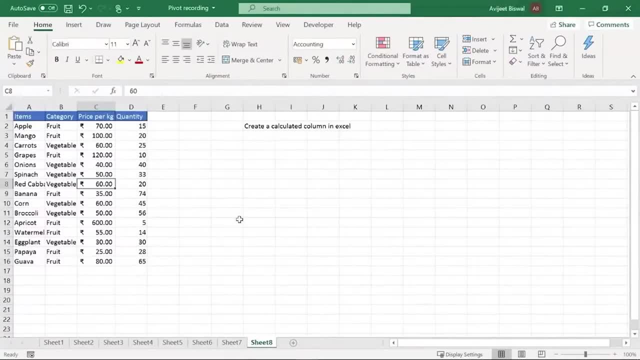 so in a pivot table you can create or use custom formulas to create calculated fields or items. calculated fields are formulas that can refer to other fields in the pivot table. calculated fields appear with other value fields in the pivot table like other value fields. a calculated fields name may proceed with. 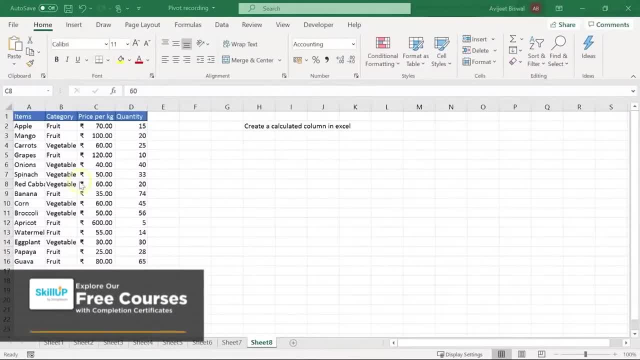 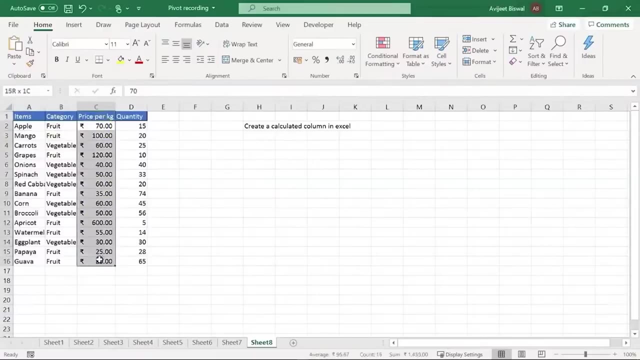 sum of followed by the field name. so here we have a sales table that has columns like the items, which has different fruits and vegetables and those have been categorized as fruits and vegetables. we have the price per kg, and this is in terms of rupees, and we have the quantity that was sold. 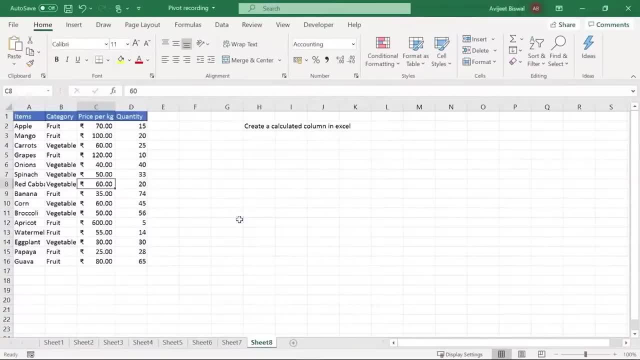 i'll tell you how you can create a calculated field or a calculated column in excel with the help of a pivot table. so in a pivot table you can create or use custom formulas to create calculated fields or items. calculated fields are formulas that can refer to other fields in the pivot. 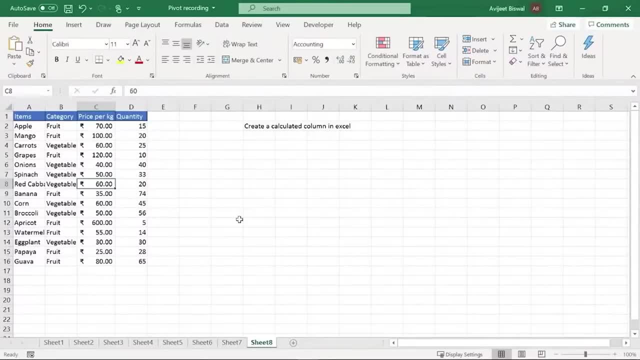 table. calculated fields appear with other value fields in the pivot table. like other value fields, a calculated fields name may proceed with sum of followed by the field name. so here we have a sales table that has columns like the item which has different fruits and vegetables and those 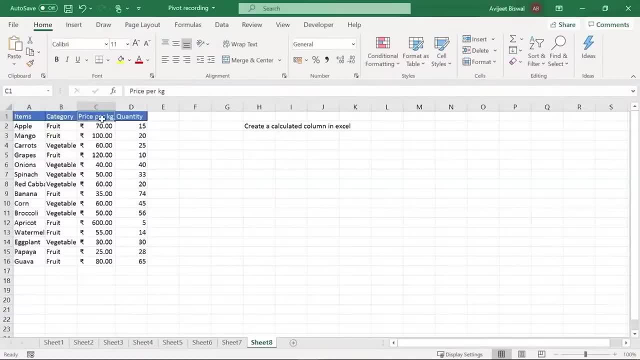 have been categorized as fruits and vegetables. we have the price per kg, and this is in terms of rupees, and we have the quantity that was sold. now let's see. if you want to find the sales for each item in the table, you can create a calculated field. 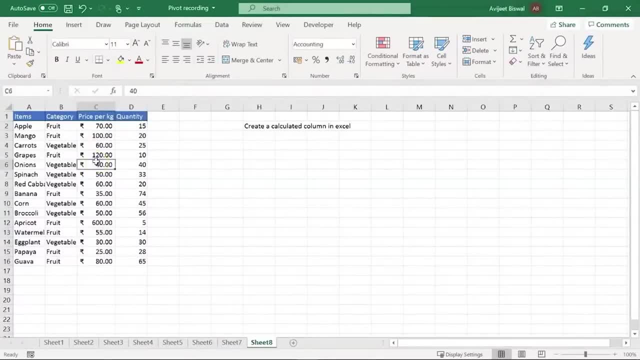 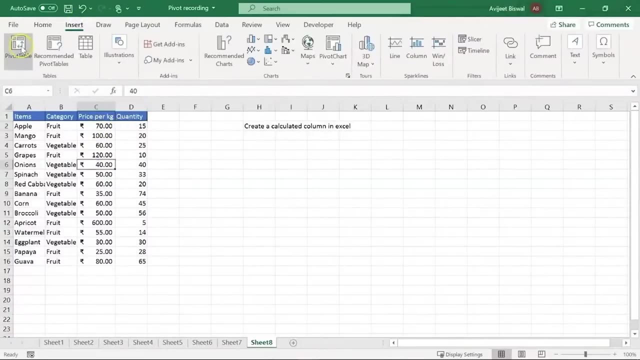 now let's see. if you want to find the sales for each item in the table, you can create a calculated field, so your sales column is going to be the product of price per kg and quantity. so let me show you how you can do that with the help of a pivot table. 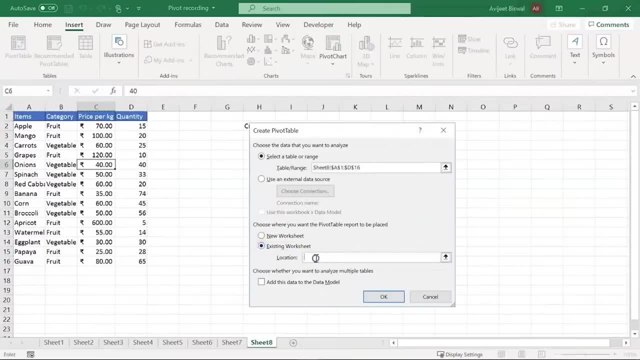 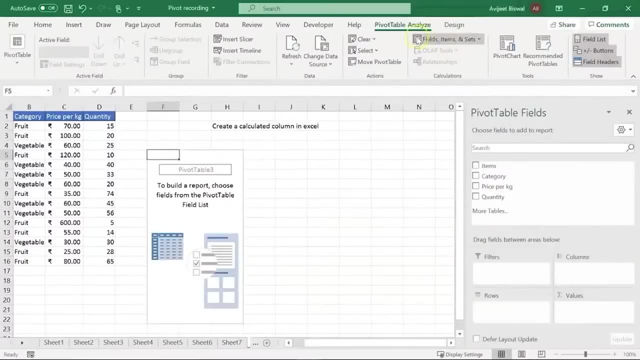 i'll create a pivot table. first, click on an empty cell, hit ok. now if you see on the top, under pivot table analyze and under calculations we have the option fields, items and sets. if i click on this drop down i get the option to create a calculated field or insert a. 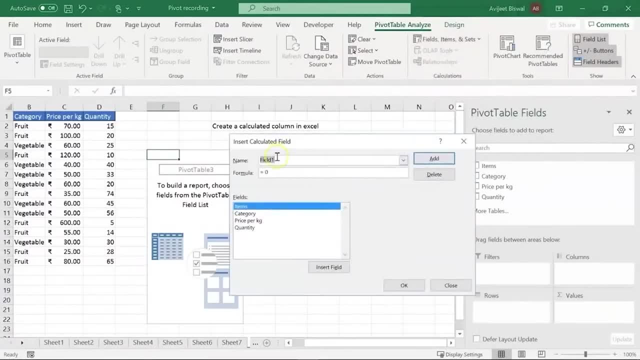 calculated field. i click on this, i'll give my field name as sales and i'll select my formula. i'll first click on price per kg and hit insert field. i'll give a space, hit shift 8 to give the product symbol and then i'll double click on. 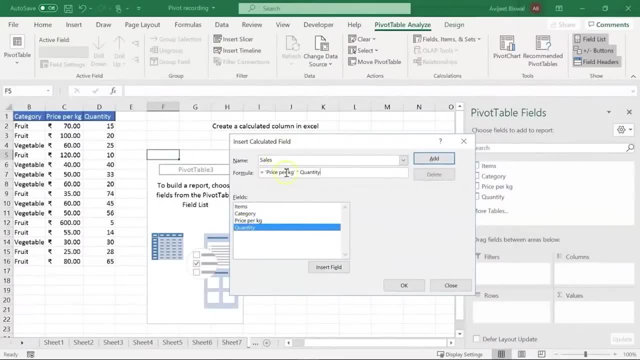 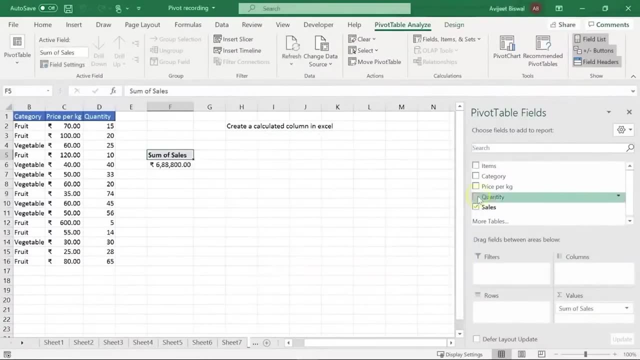 quantity. now this is my formula for sales, that is, price per kg multiplied by quantity. i'll click on add and i click on ok. if you see here there is a calculated field that is present in the pivot table fields, which is sales, but it did not add it to. 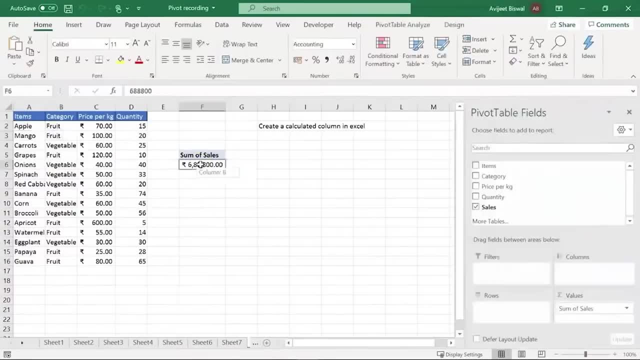 our original table. our original table is the same, but here we have added a calculated field which is present only in the pivot table list. now we can use this. it has already taken it under values. now let's say i want to find the sum of sales for 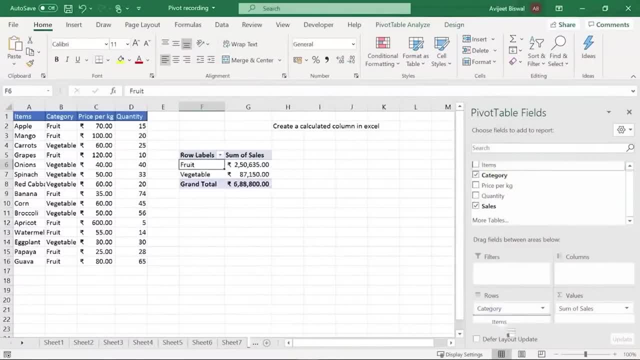 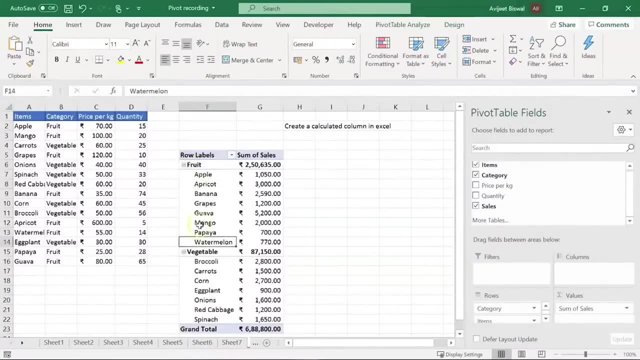 each item under each category. you can see it here: we have our category fruit and we have our category vegetable, and under that we have different items like apple, apricot, banana. similarly, in vegetables we have broccoli, carrots, corn, eggplant and others. so this is how you can create a calculated. 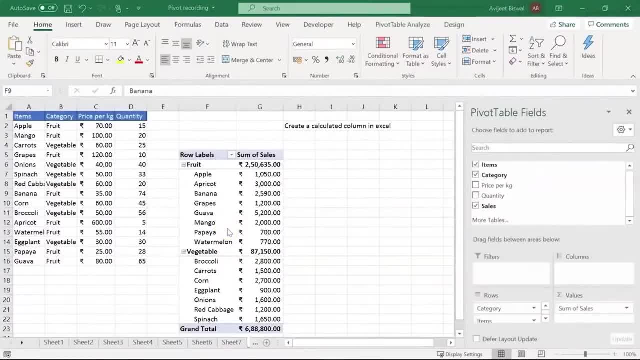 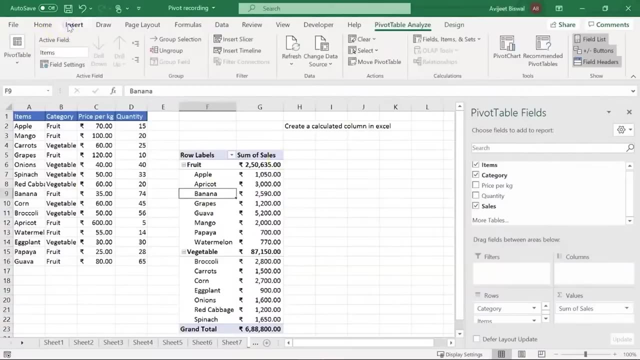 field in a pivot table. now, this one more good feature that excel offers us in pivot table is to create a pivot chart, so you can use your pivot table and create different charts. so i'll show you how to do that. if i go to insert here, i have the option of: 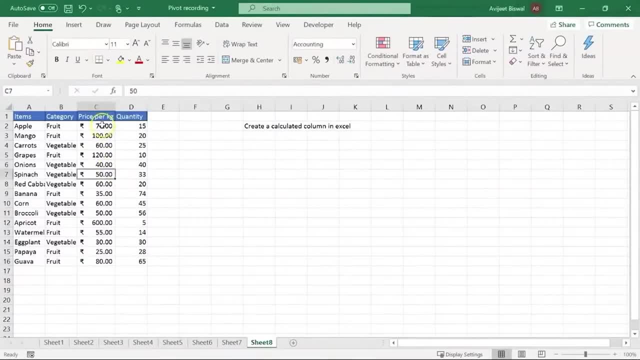 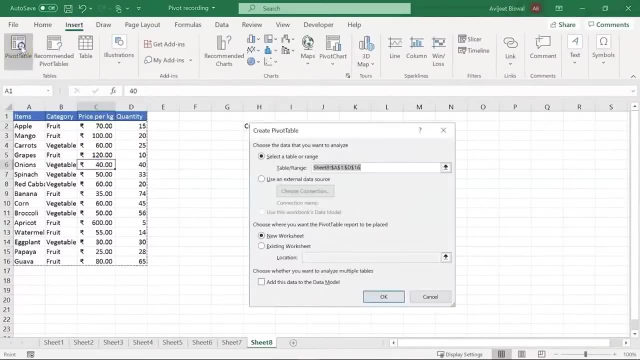 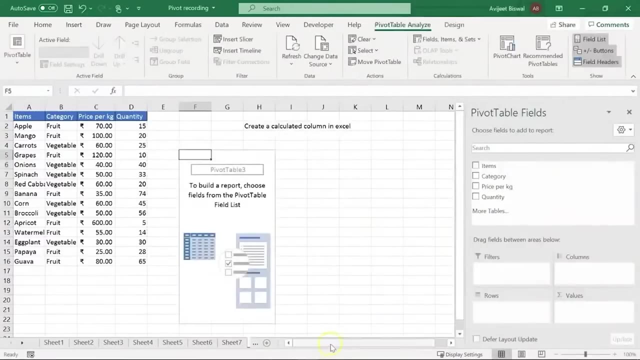 so your sales column is going to be the product of price per kg and quantity. so let me show you how you can do that with the help of a pivot table. I will create a pivot table. first, click on an empty cell. hit ok. now, if you see on the top, 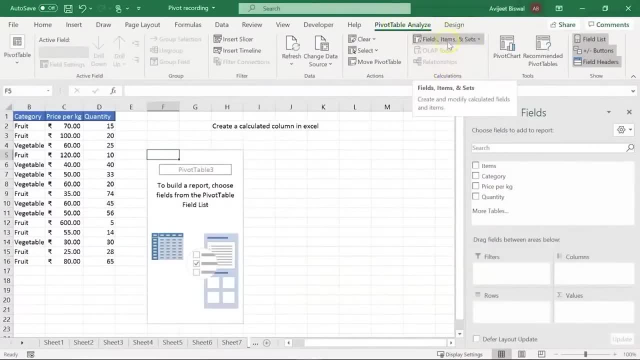 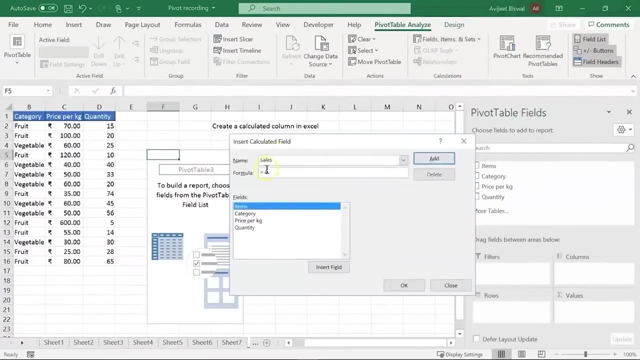 under pivot table, analyze and under calculations, we have the option fields, items and sets. if I click on this drop down, I get the option to create a calculated field or insert a calculated field. I click on this, I will give my field name as sales and I will select. 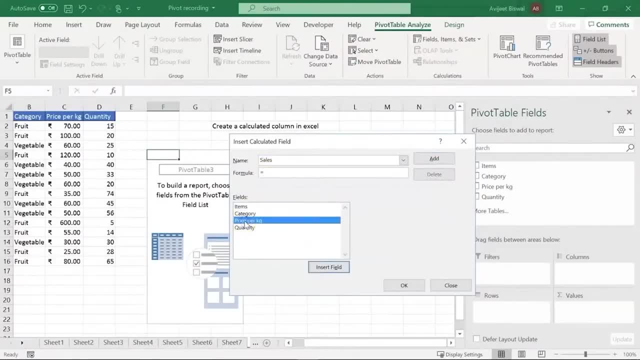 my formula. I will first click on price per kg and hit insert field. I will give a space, hit shift 8 to give the product symbol and then I will double click on quantity. now this is my formula for sales, that is, price per kg multiplied by quantity. 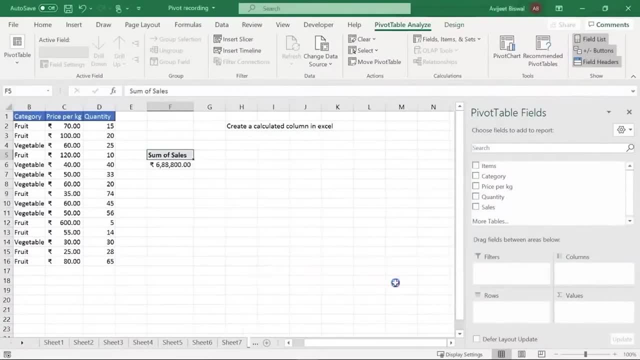 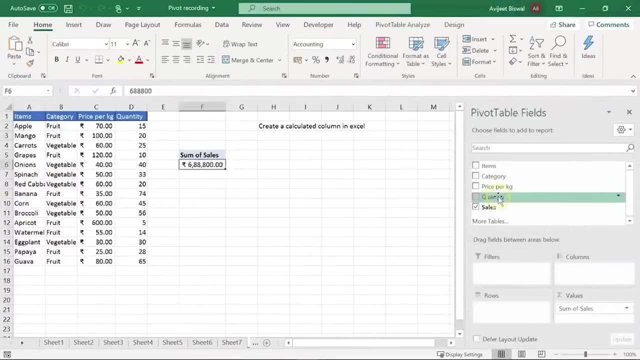 I will click on add and I click on ok. if you see, here there is a calculated field that is present in the pivot table fields, which is sales, but it did not add it to our original table. our original table is the same, but here we have added a calculated. 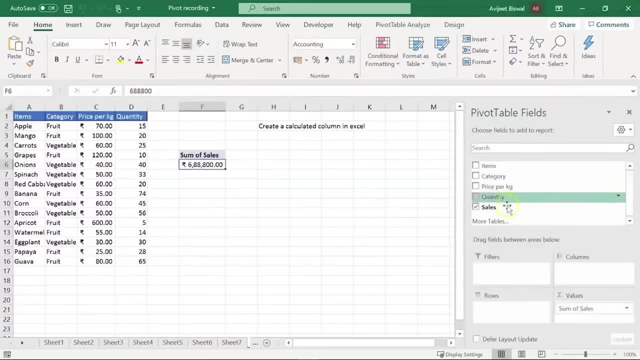 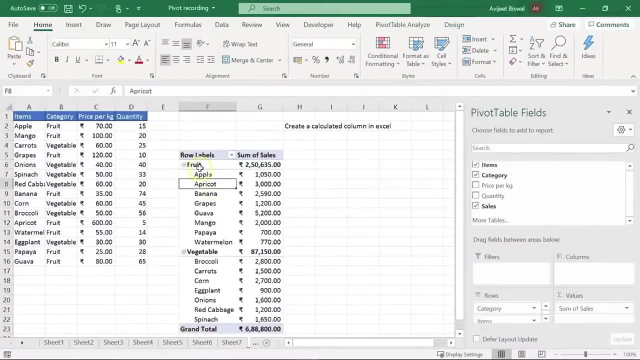 field which is present only in the pivot table list. now we can use this. it has already taken it under values. now let's say I want to find the sum of sales for each item under each category. you can see it here. we have our category fruit and 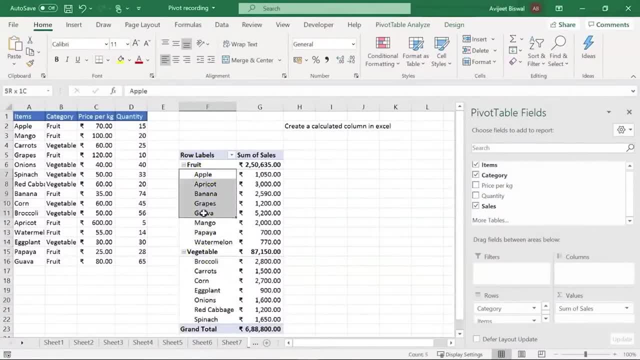 we have our category vegetable and under that we have different items like apple, apricot, banana. similarly, in vegetables we have broccoli, the carrots, corn, eggplant and others. so this is how you can create a calculated field in a pivot table. now this one more good feature that excel offers. 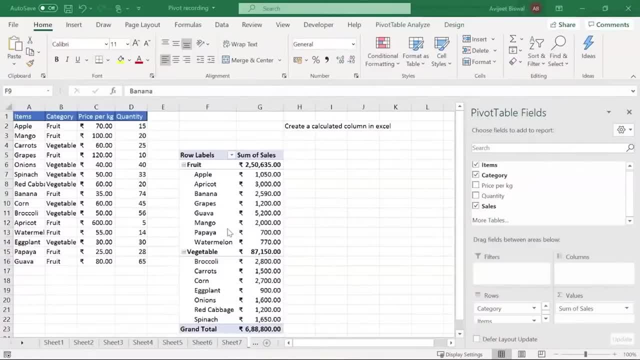 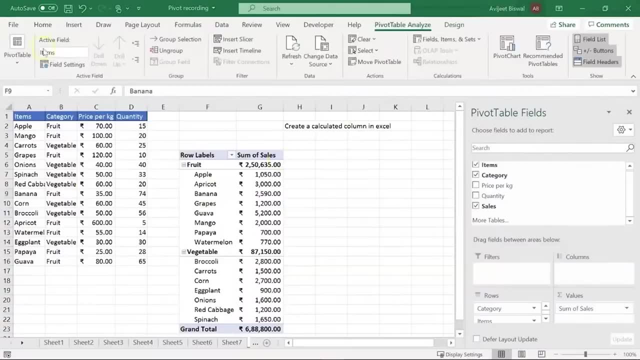 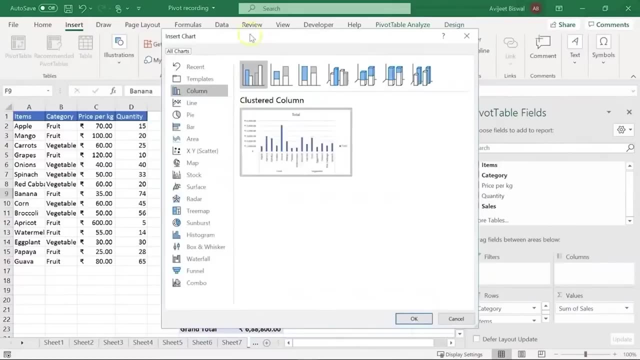 us in pivot table is to create a pivot chart so you can use your pivot table and create different charts. so I will show you how to do that. if I go to insert here, I have the option of recommended charts. click on this. excel gives me some default charts. 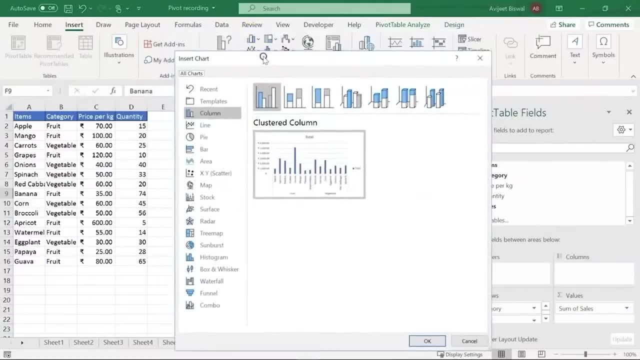 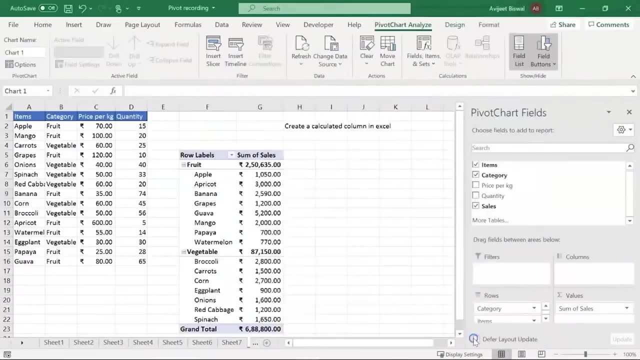 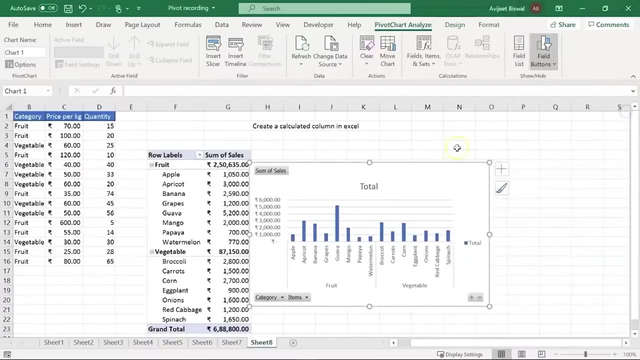 recommended charts. click on this. excel gives me some default charts which you can use. let's say i'll select this. let me drag it a bit to the right here you can see i'll close this pivot field list. this is a nice bar chart that excel has created. this is called a. 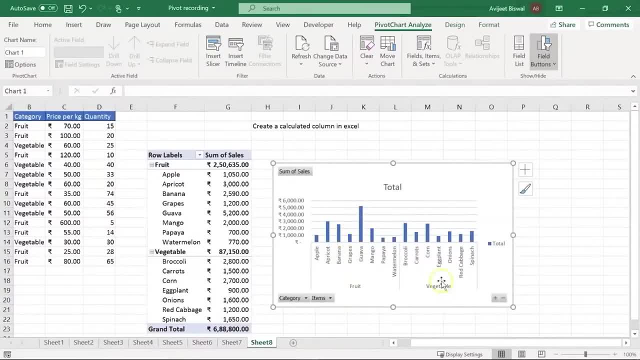 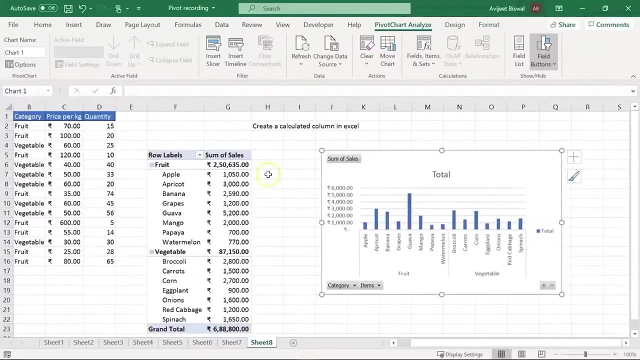 pivot chart. now here you can see the category fruits and vegetables and the different fruits and vegetables or the items. in the y-axis you can see the total sales. if you see from the graph, guava made the highest amount of sales. now, if i sort this, let's sort. 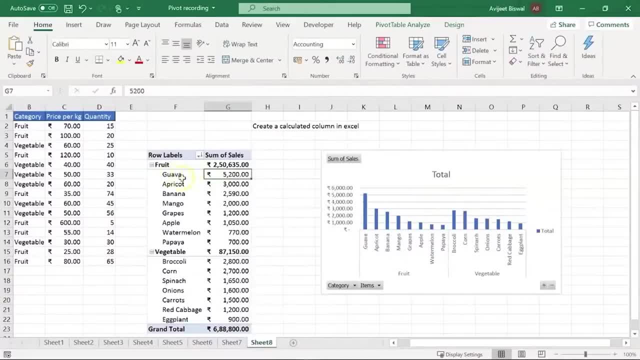 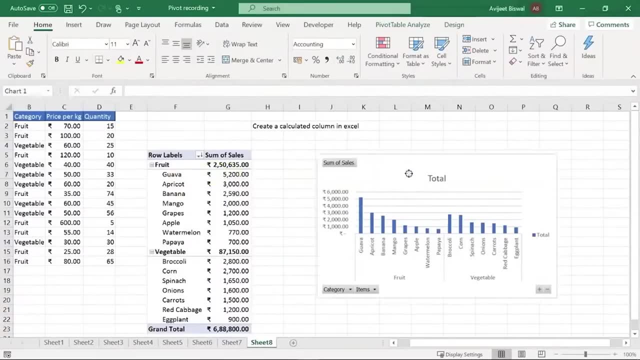 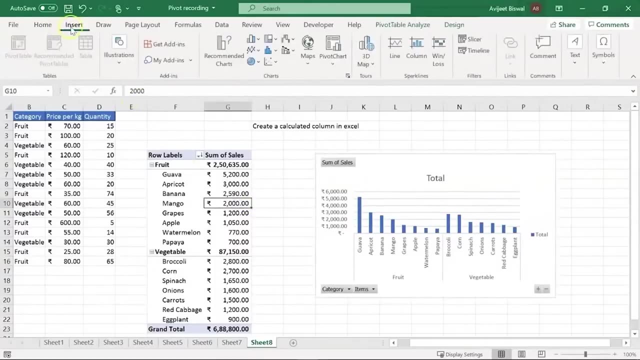 this first. you can see it here: fruit guava made the highest amount of sales. now, since i sorted and changed my pivot table, the pivot chart also automatically gets updated. similarly, there are other charts also that you can create. let's go to the insert tab and let's 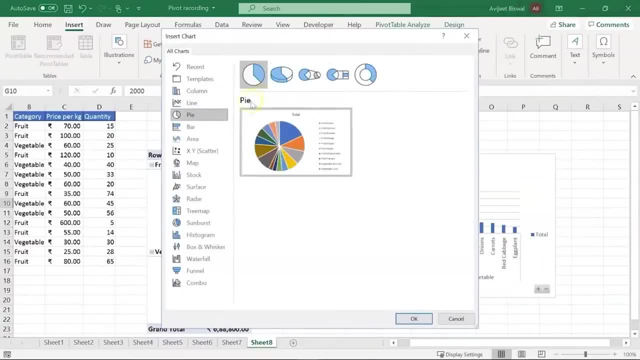 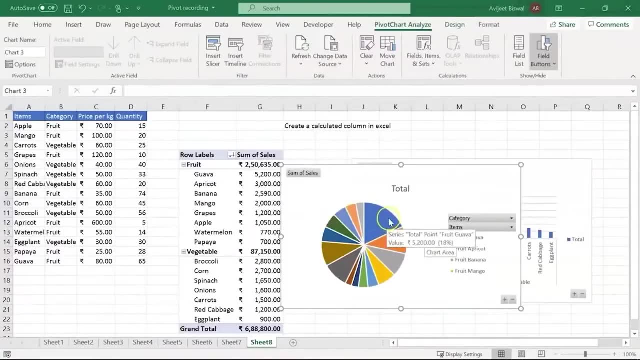 click on recommended charts again. let's look for a pie chart. so this is a pie chart that you can create. let me click on ok, so here is our pie chart and each pie represents a certain item and the pie that has the highest area represents it had the highest amount of sales. 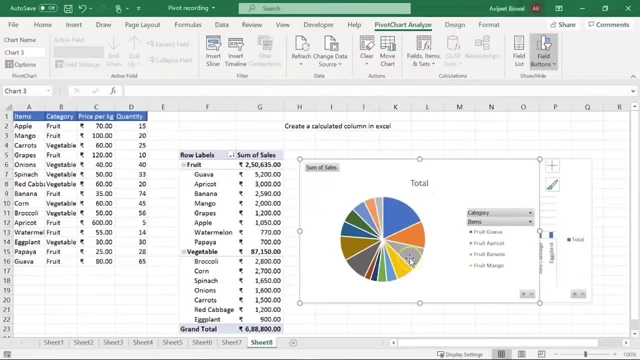 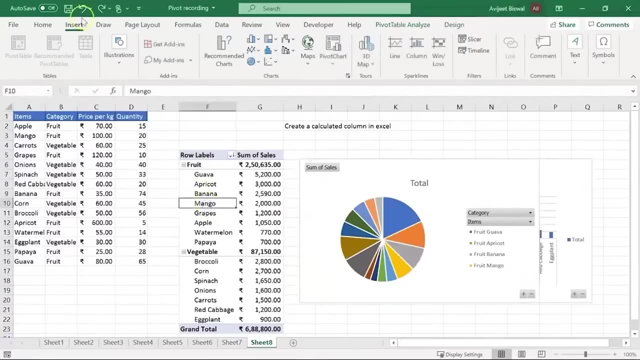 in this case you can see it is guava, and similarly we have other items as well. this is fruit, banana, that's corn, and we have spinach and others. let's explore a few other charts. so first i'll click on my pivot table, go to insert and under recommended charts, let's 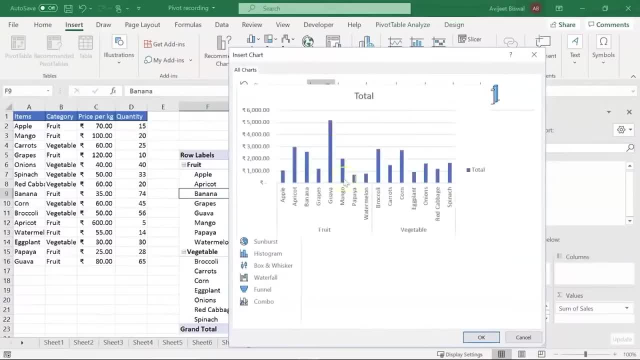 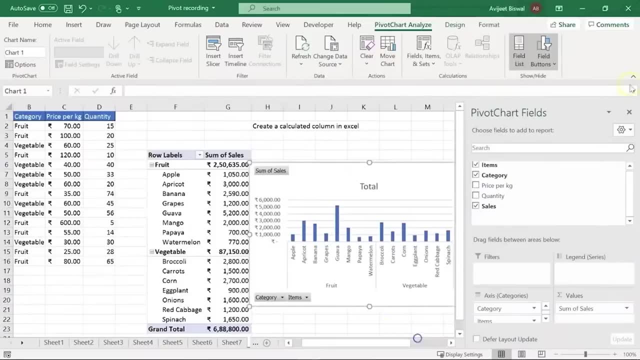 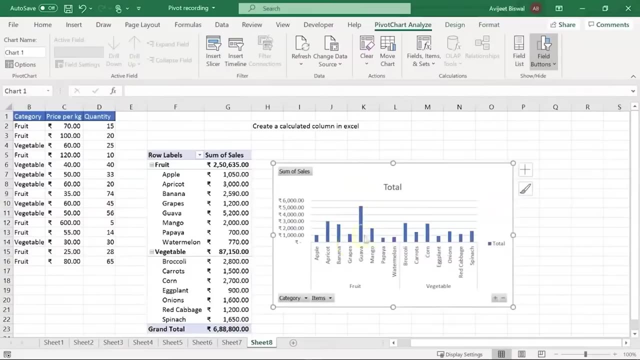 which you can use. let's say I will select this. let me drag it a bit to the right. here you can see I will close this pivot field list. this is a nice bar chart that excel has created. this is called a pivot chart. now, here you can see. 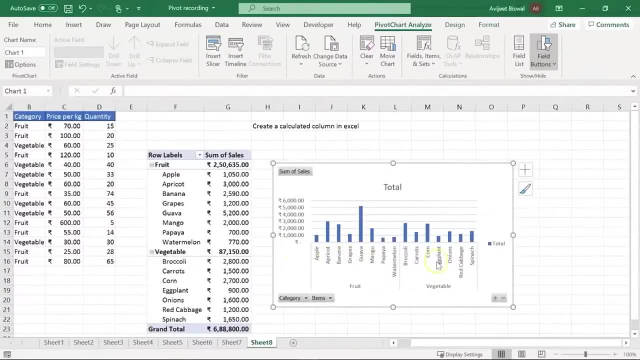 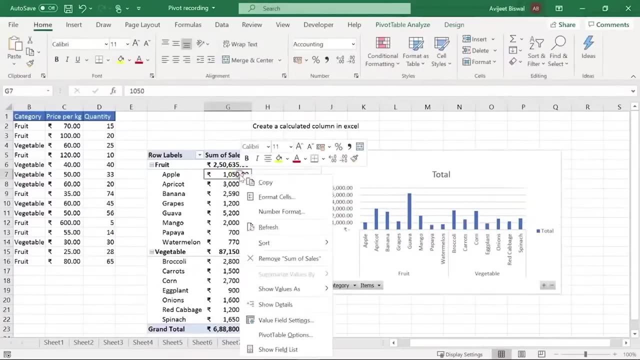 the category fruits and vegetables and the different fruits and vegetables or the items in the y axis, you can see the total sales. if you see from the graph, guava meet the highest amount of sales. now, if I sort this, let's sort this first. you can see it. 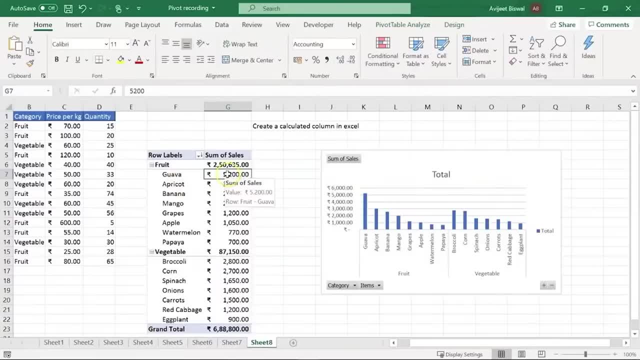 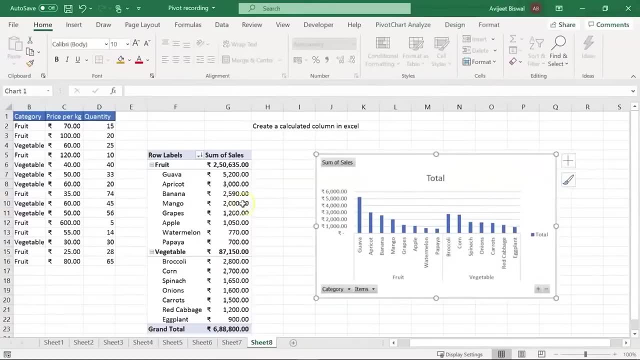 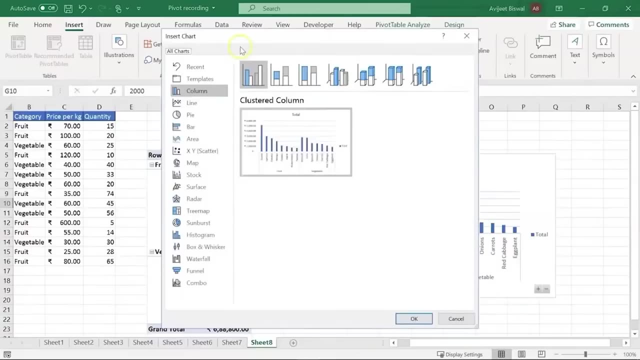 here, fruit guava meet the highest amount of sales. now, once I sorted and changed my pivot table, the pivot chart also automatically gets updated. similarly, there are other charts also that you can create. let's go to the insert tab and let's click on recommended charts again. let's look for. 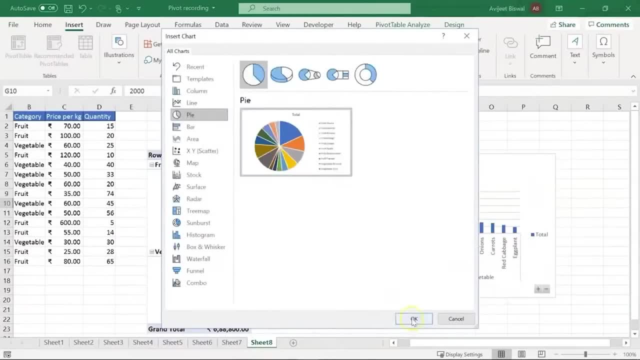 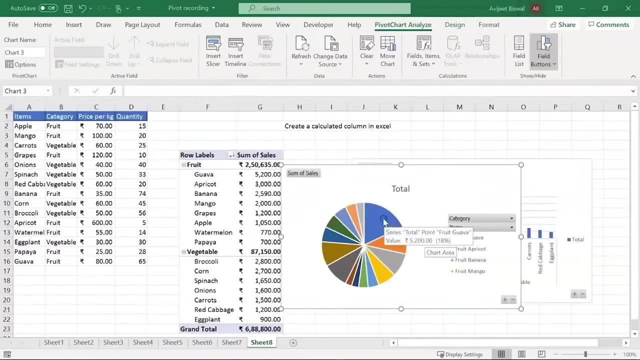 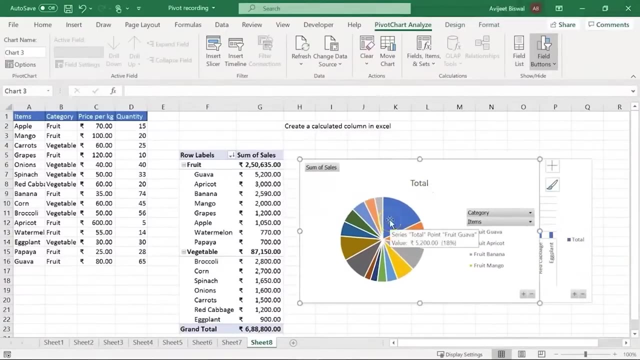 a pie chart. so this is a pie chart that you can create. let me click on ok. so here is our pie chart, and each pie represents a certain item and the pie that has the highest area represents it had the highest amount of sales in this case. you can see: 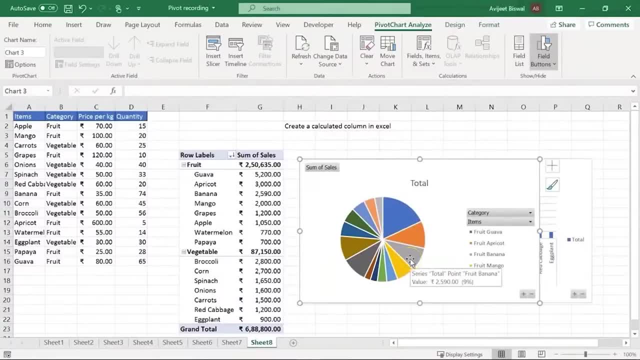 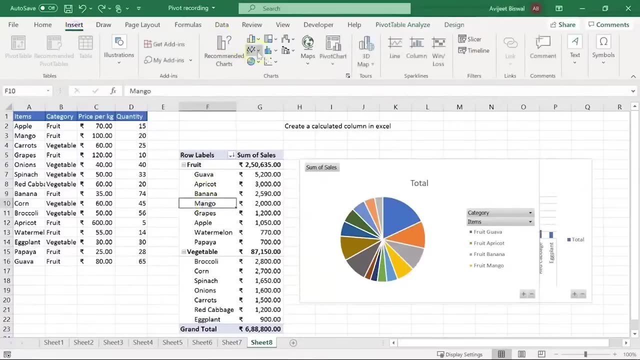 it is guava, and similarly we have other items as well. this is fruit, banana, that's corn, and we have spinach and others. let's explore a few other charts. so first I'll click on my pivot table, go to insert and under recommended charts let's now select a. 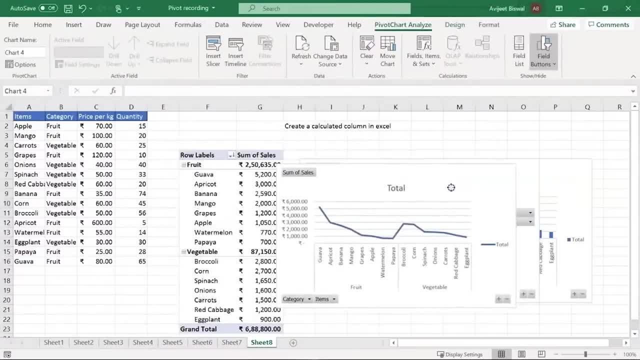 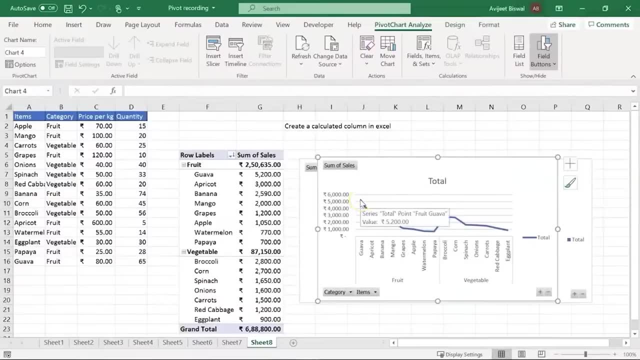 line chart. if I hit ok, move it to the right. so this is a line chart. you can see it starts from guava, which had the highest amount of sales, then it drops and in the x axis you can see the different items. similarly, when it starts with the vegetables, 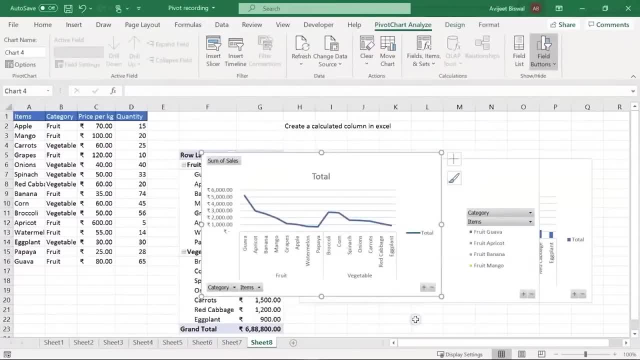 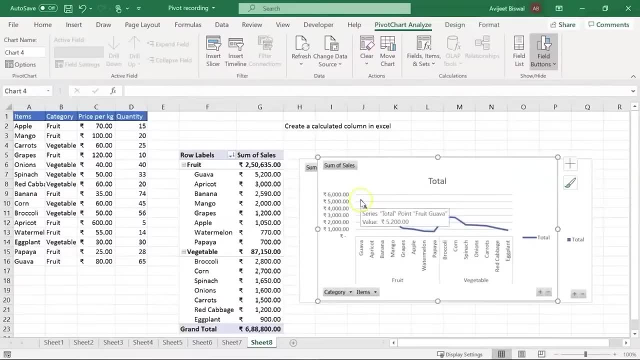 now select a line chart. if i hit ok, move it to the right. so this is a line chart. you can see it starts from guava, which had the highest amount of sales, then it drops and in the x axis you can see the different items. similarly, when it starts with the vegetables, 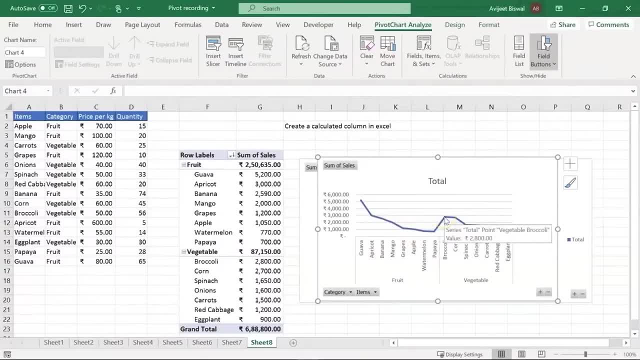 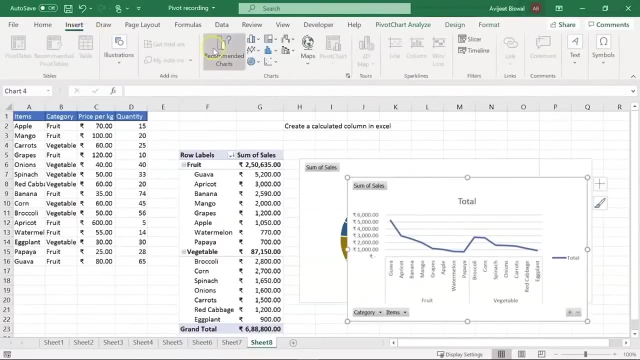 brocoli made the highest amount of sales with 2800 rupees and our lowest was eggplant at 900 rupees. for fruits, papaya sold the least at 700 rupees. let's take another chart i'll go to insert under recommended charts. let's see. 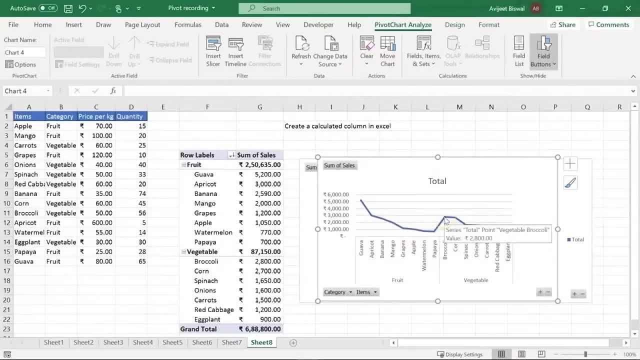 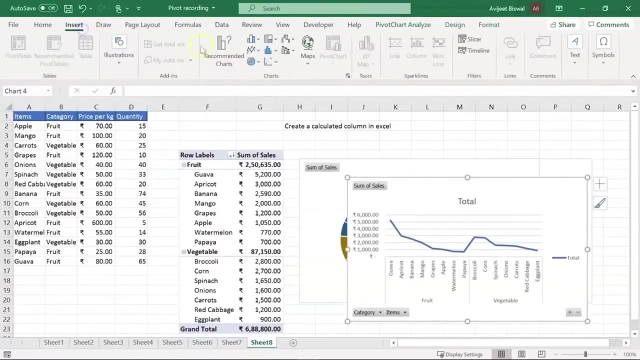 brocoli made the highest amount of sales with 2800 rupees and our lowest was eggplant at 900 rupees. for fruits, papaya sold the least at 700 rupees. let's take another chart I'll go to insert under recommended charts. let's: 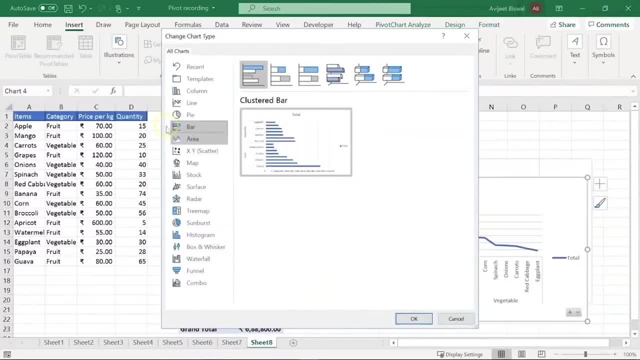 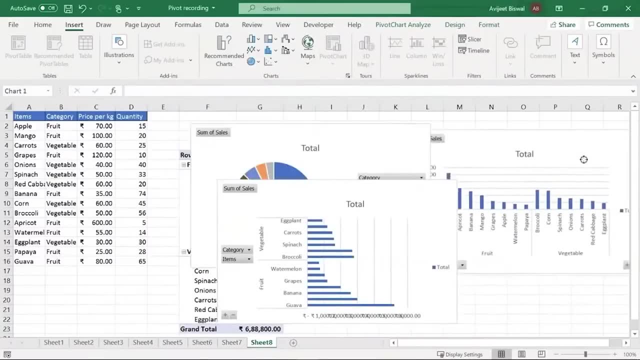 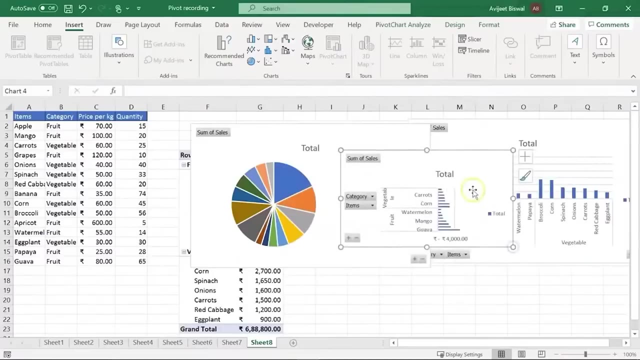 see. this time we'll see a bar chart. now this is a horizontal bar chart and not a vertical one. we just saw a vertical column chart like this. this is an horizontal bar chart. now you can always increase and decrease the size of these charts. let's explore. 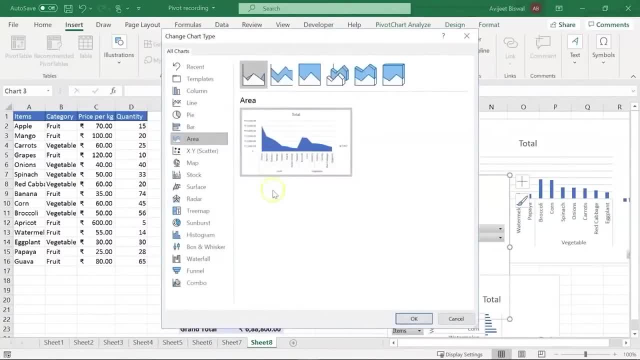 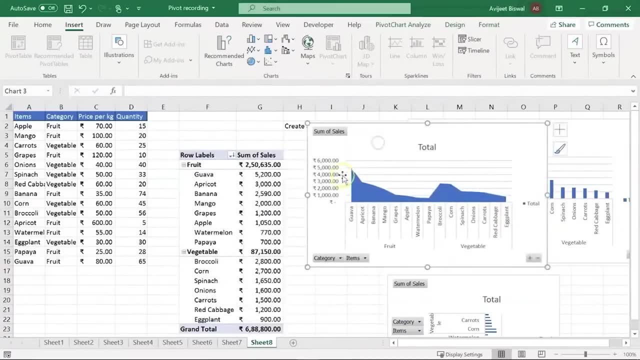 a last chart. let's take the area chart for now. so this is an area chart. again, it looks similar to the line chart. it starts with guava, which had the highest amount of sales. similarly, papaya, under fruits, had the lowest amount of sales. under vegetables, it was. 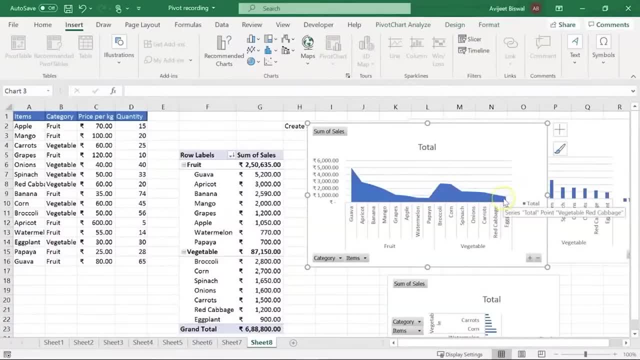 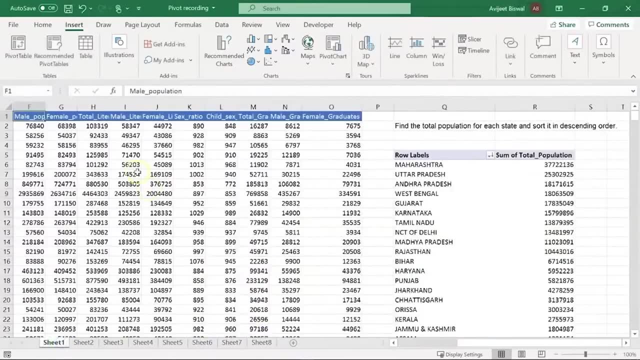 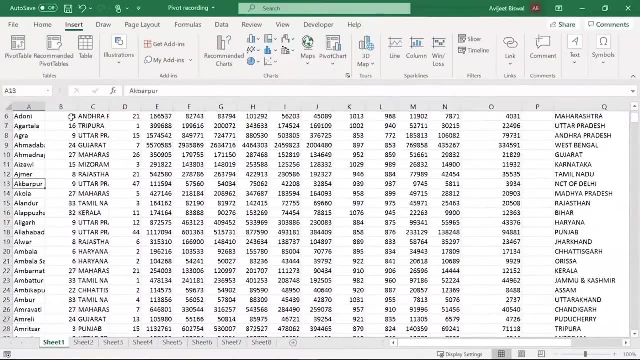 brocoli and, finally, eggplant made the lowest amount of sales under vegetables. now let's go to our first sheet and summarize what we have done in this demo. what we have done is we have created pivot tables in excel, so we had our data. this is 2011 census data. 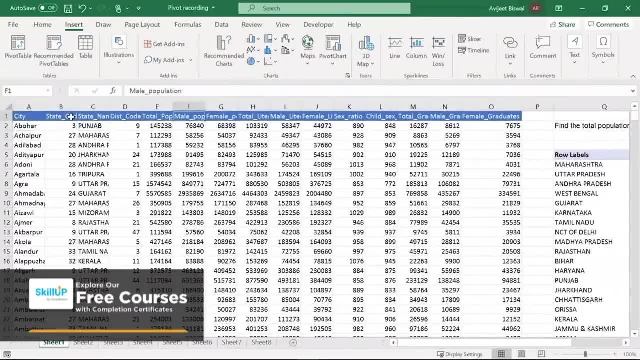 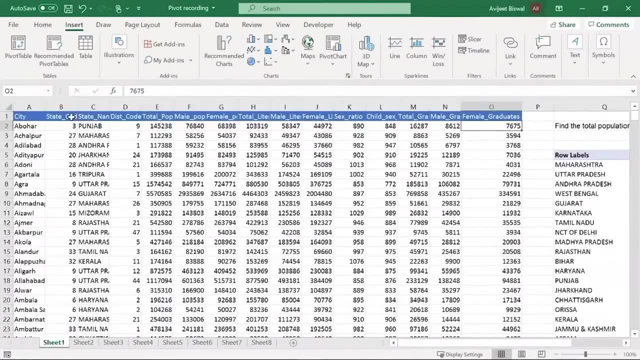 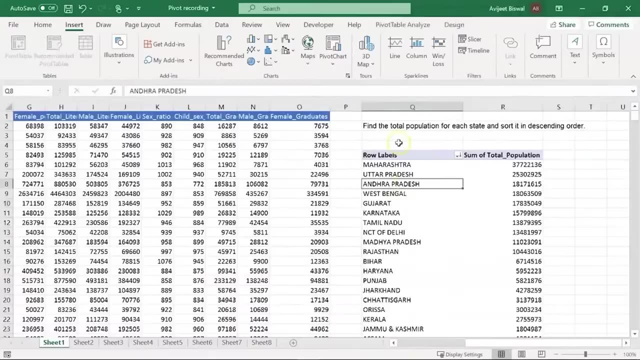 from india. we had the different cities, the state names and we had the total population: total literates, female literates, male literates. we had the sex ratio, total graduates and other information. so we began by understanding how to create a simple pivot table where we calculated the 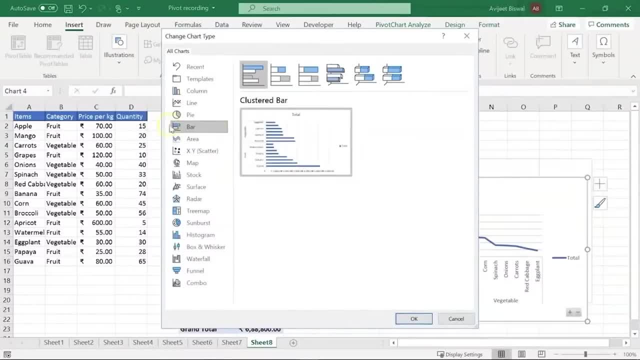 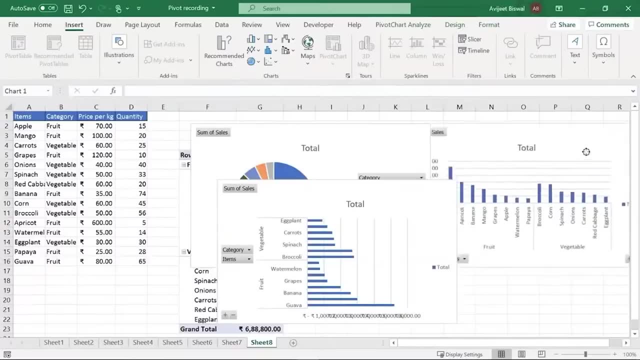 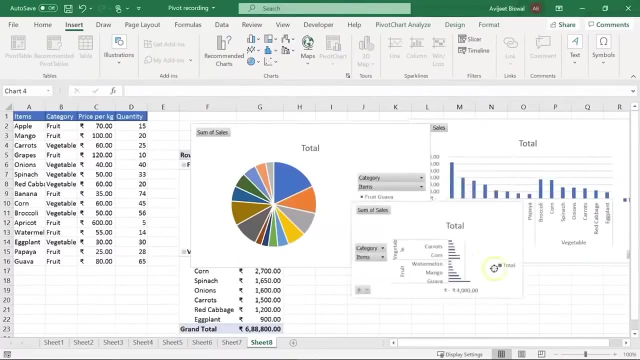 this time we'll see a bar chart. now, this is a horizontal bar chart and not a vertical one. we just saw a vertical column chart like this: this is an horizontal bar chart. now you can always increase and decrease the size of these charts. let's explore a last chart. let's 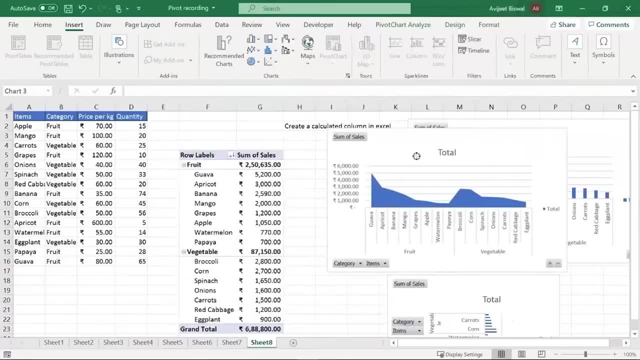 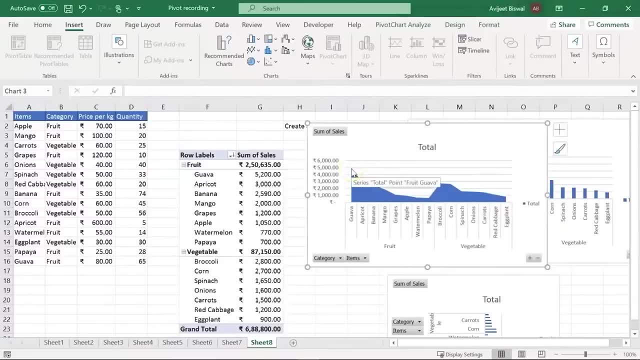 take the area chart for now. so this is an area chart. again, it looks similar to the line chart. it starts with guava, which had the highest amount of sales. similarly, papaya, under fruits, had the lowest amount of sales. under vegetables, it was brocoli and finally eggplant made the lowest amount of sales. 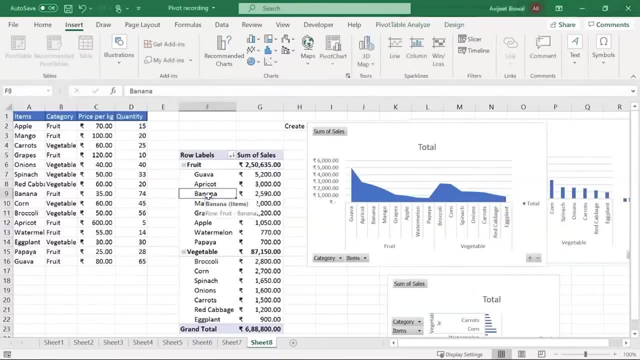 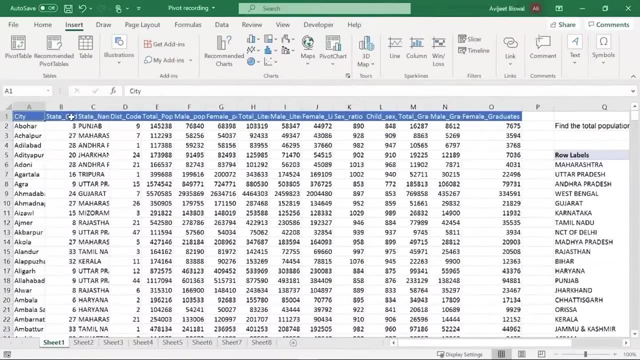 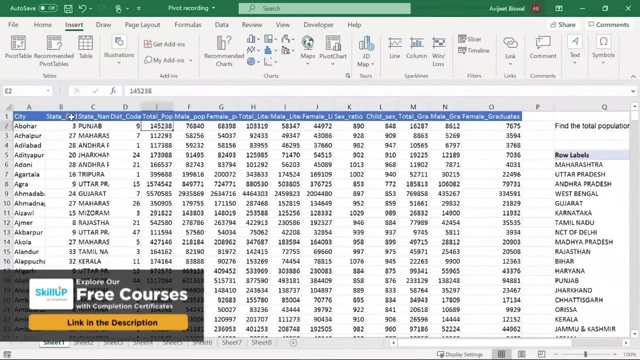 under vegetable. now let's go to our first sheet and summarize what we have done in this demo for pivot tables in excel. so we had our data. this is 2011 census data from india. we had the different cities, the state names and we had the total population. 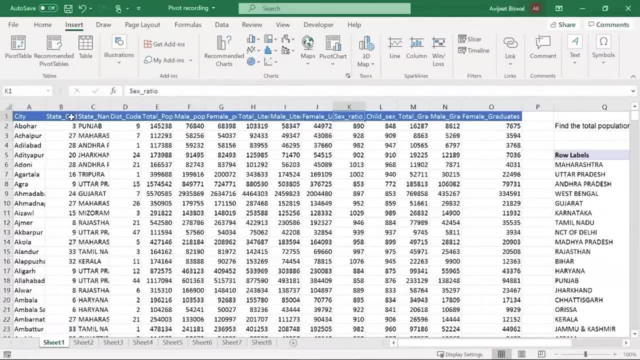 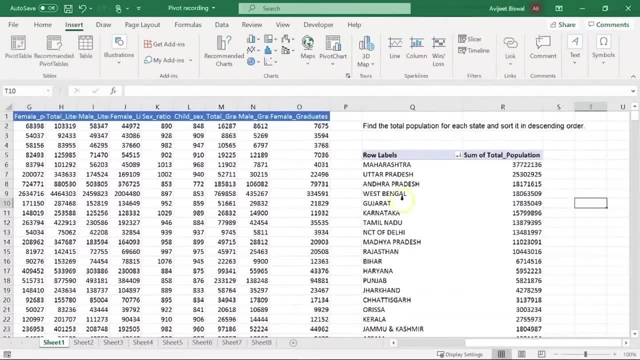 total literates, female literates, male literates. we had the sex ratio, total graduates and other information, so we began by understanding how to create a simple pivot table where we calculated the total population for each state and sorted it in descending order. we found that maharashtra. 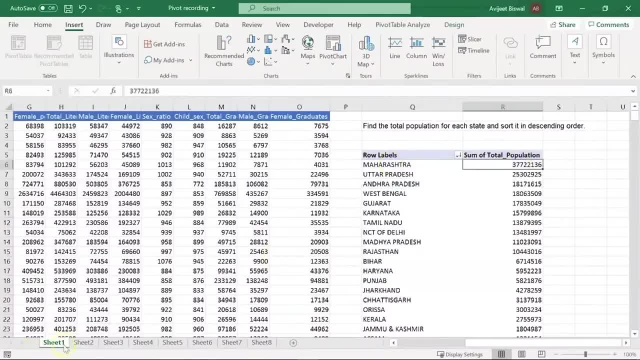 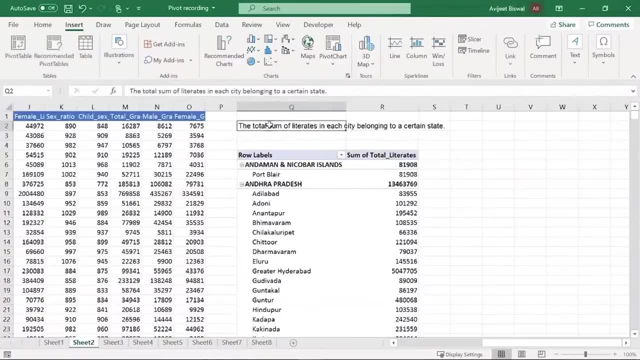 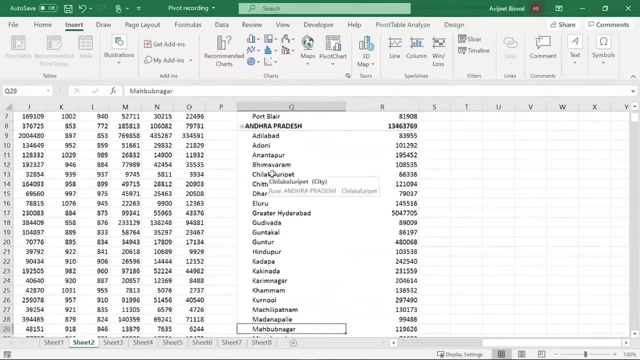 uttar pradesh had the total population in 2011. then we saw another pivot table where we calculated the total sum of literates in each city belonging to a certain state. so you can see we had the different state names and the cities under each state. 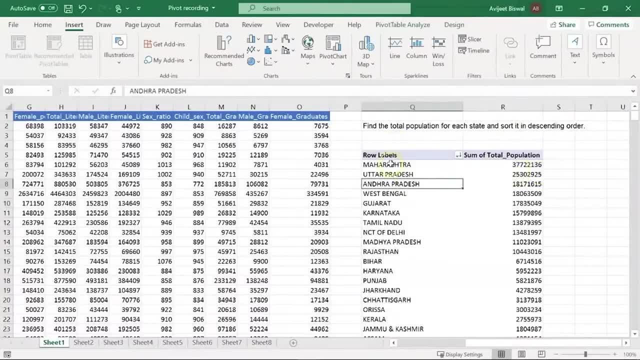 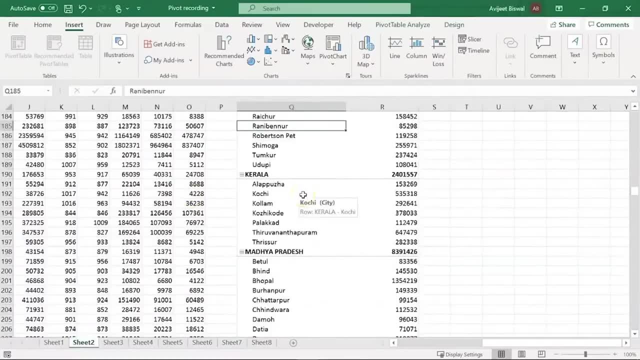 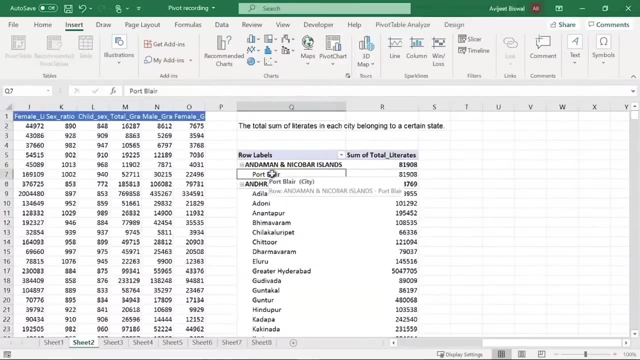 total population for each state and, ending order, we found that maharashtra, uttar pradesh, had the total population in 2011. then we saw another pivot table where we calculated the total sum of literates in each city belonging to a certain state. so you can see, we had the. 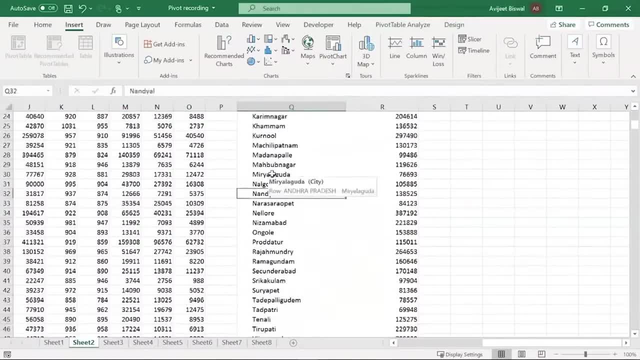 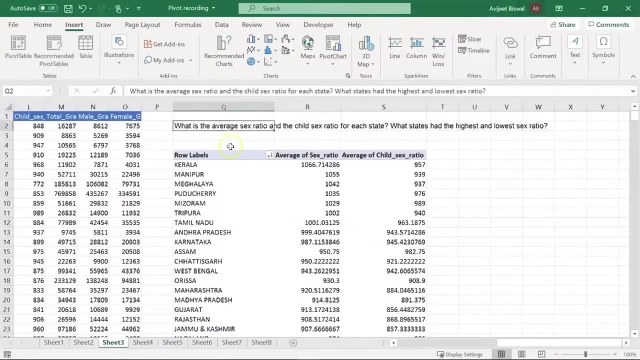 different state names and the cities under each state. then we saw another feature where you could calculate the average of a certain numerical column. so here we calculated the average sex ratio and the child sex ratio for each state and found out which one had the highest and lowest sex ratio. 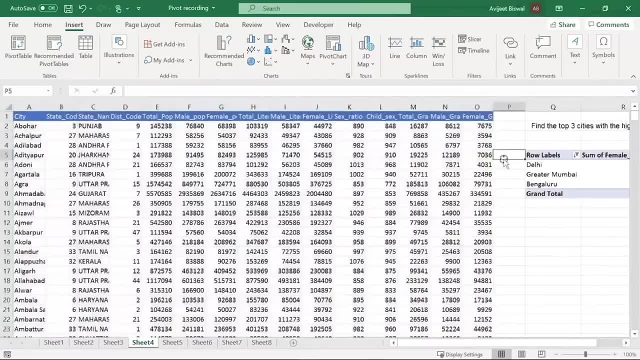 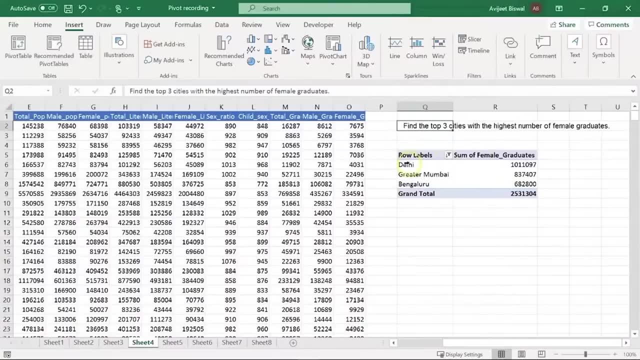 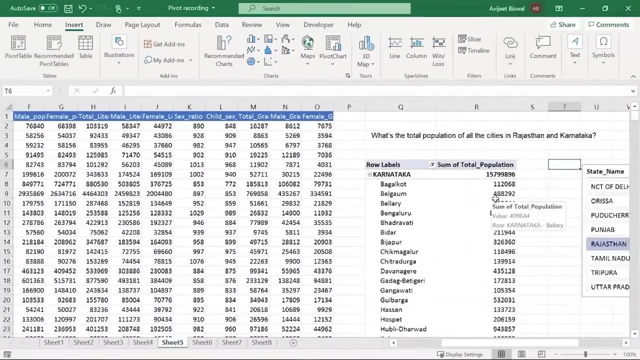 after that, we saw how you could find or filter tables. we saw how to find the top three cities with the highest number of female graduates. we found out that delhi, greater mumbai and bangalore were the top cities with highest number of female graduates. next, we saw how to use 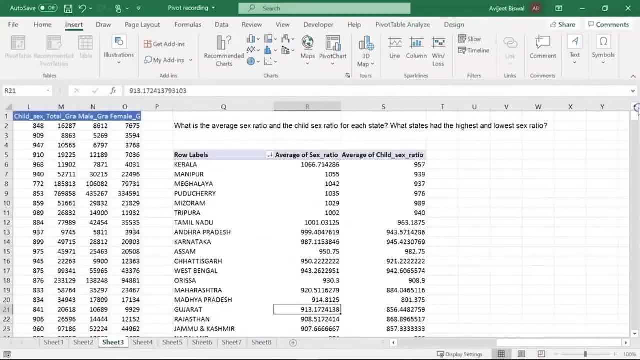 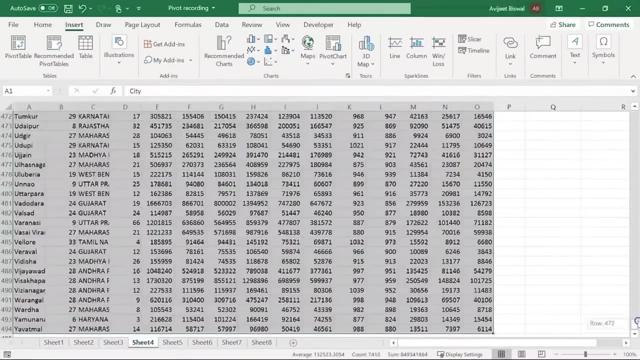 then we saw another feature where you could calculate the average of a certain numerical column. so here we calculated the average sex ratio and the child sex ratio for each state and found out which one had the highest and lowest sex ratio. after that we saw how you could find. 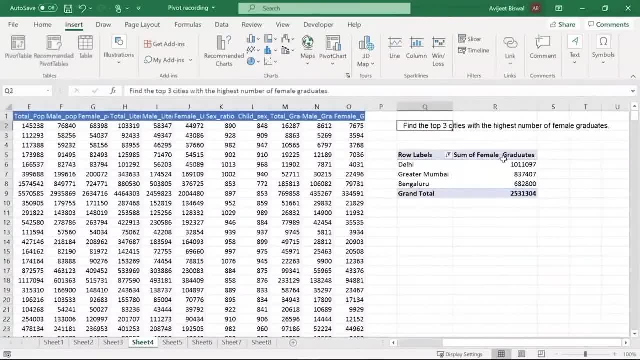 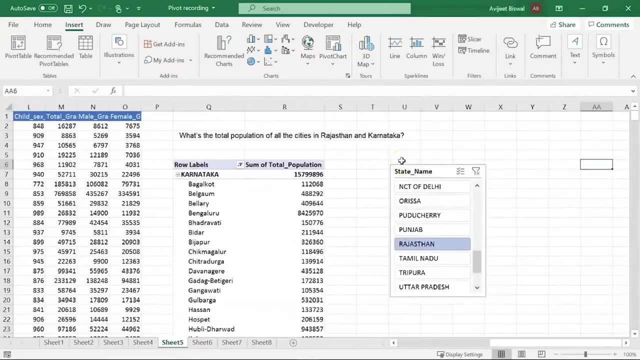 or filter tables. we saw how to find the top three cities with the highest number of female graduates. we found out that delhi, greater mumbai and bangalore with the top cities with highest number of female graduates. next, we saw how to use slicer in a pivot table, so we sliced. 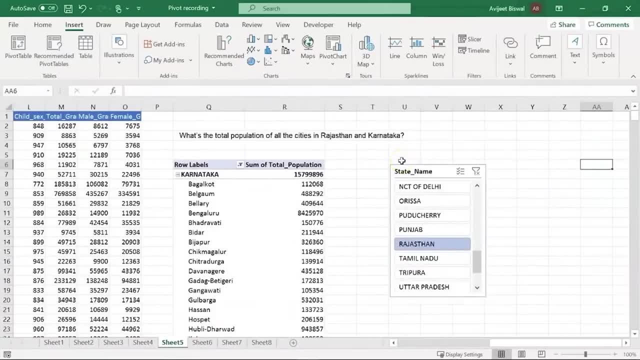 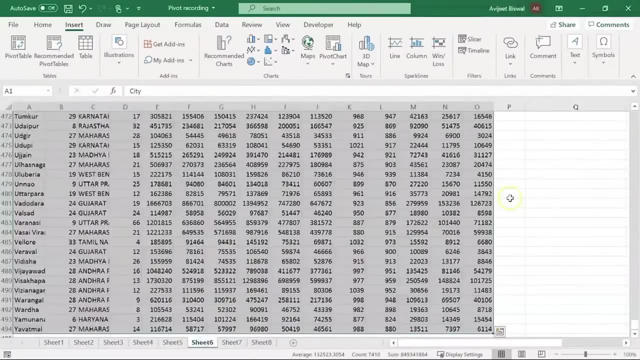 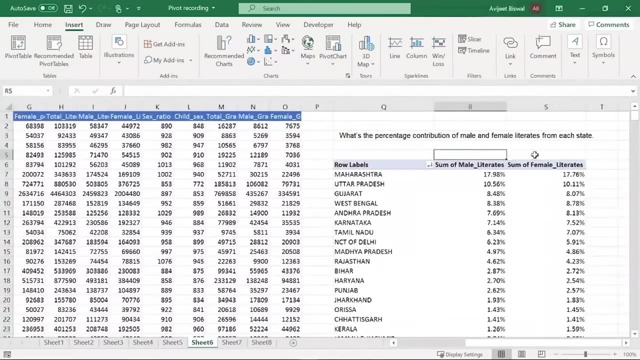 slicer in a pivot table. so we sliced our table based on rajasthan and karnataka state and saw the total population for all the cities in rajasthan and karnataka in the next sheet. we explored another feature, that was to find the percentage contribution. 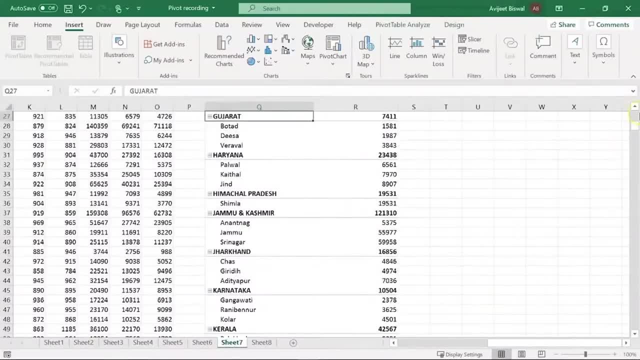 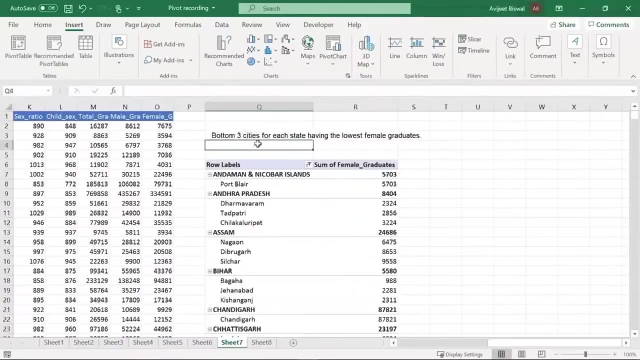 of male and female literates from each state. then here we saw how to find out the bottom three cities for each state having lowest female graduates. and one thing: we marked that some of the states did not have three cities. for example, andaman had only one city, that was sport player. 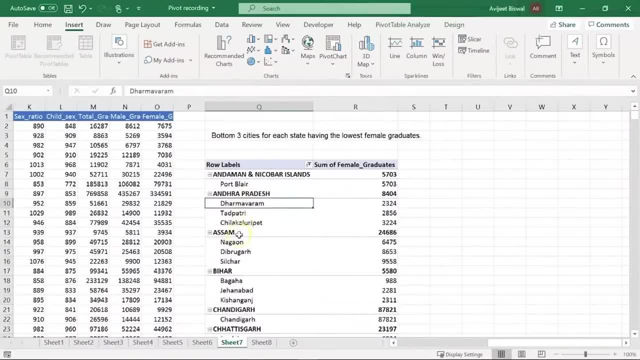 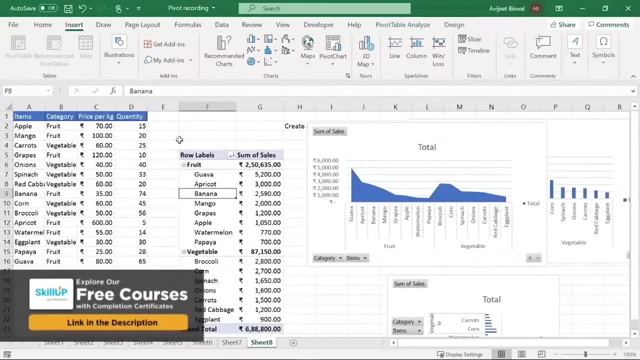 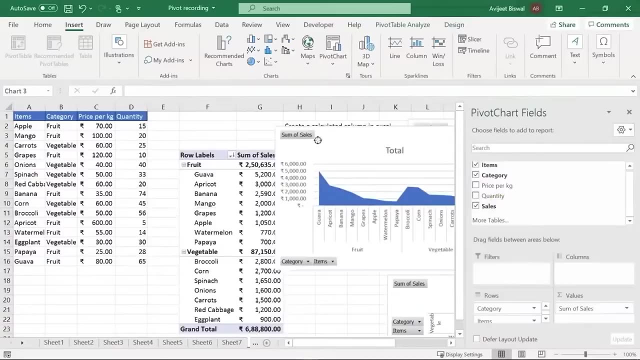 but the others. we found out the bottom three cities that had the lowest female graduates. finally, we looked at how to create a calculated field in a pivot table. so we saw how to create a calculated field called sales, and then we explored how to create different charts and graphs. so this 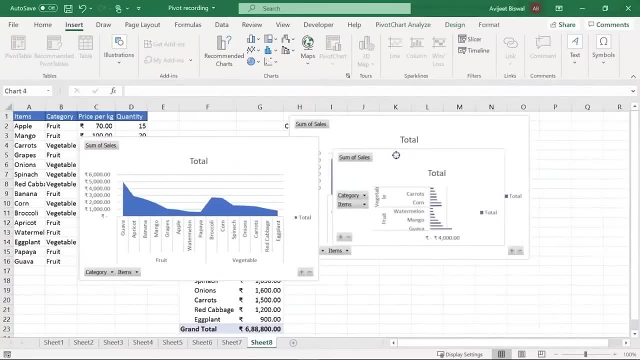 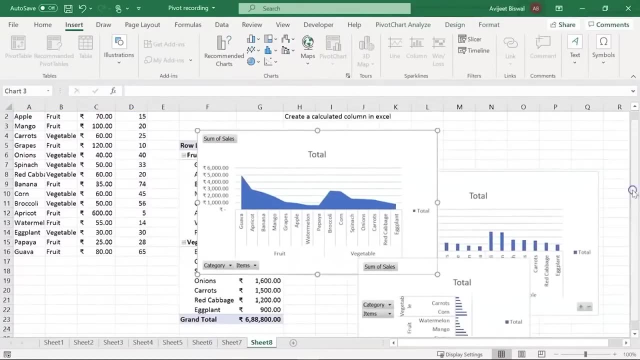 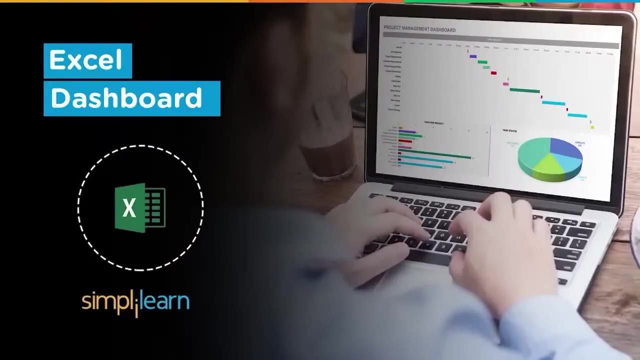 was an area chart. that we saw is a column chart. we also saw, or looked at, a bar chart. that was a horizontal bar chart. similarly, we saw how to create a pie chart as well. in this video, we will be creating two dashboards using a sample sales dataset. 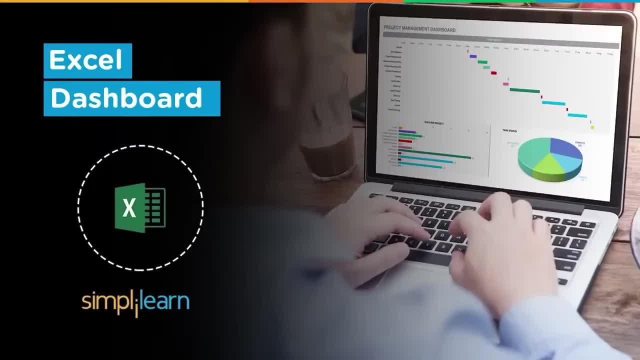 so if you want to get the data and the dashboard file that we will be creating in this demo, then please put your email ids in the comment section of the video. our team will share the files via email. now let's begin by understanding what is a dashboard in excel. 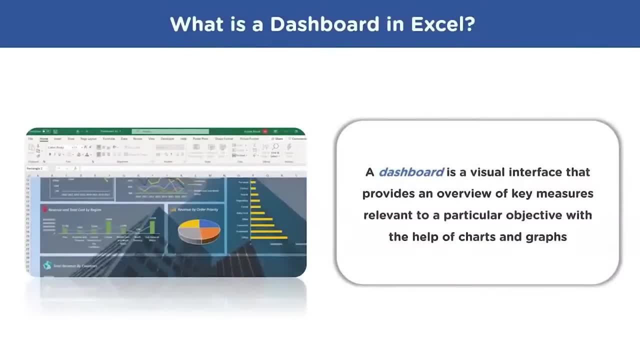 a dashboard is a visual interface that provides an overview of key measures relevant to a particular objective with the help of charts and graphs. dashboard reports allow managers to get a high level overview of the business and help them make quick decisions. there are different types of dashboards, such as strategic dashboards. 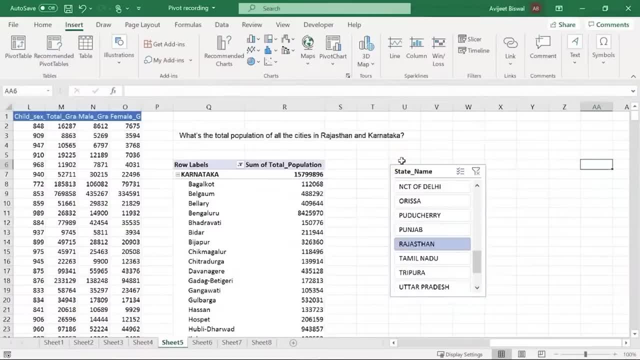 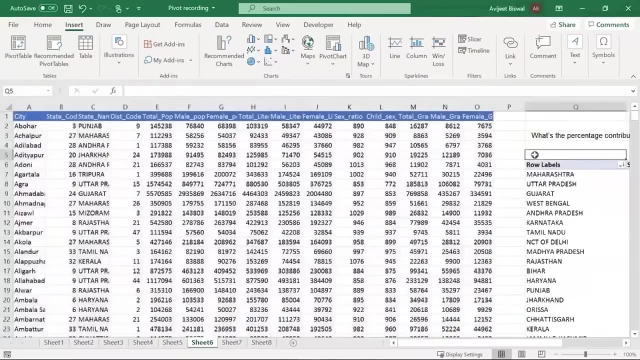 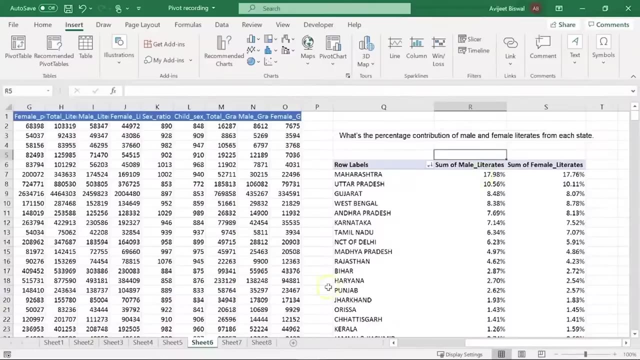 our table based on rajasthan and karnataka state and saw the total population for all the cities in rajasthan and karnataka. in the next sheet we explored another feature that was to find the percentage contribution of male and female literates from each state. 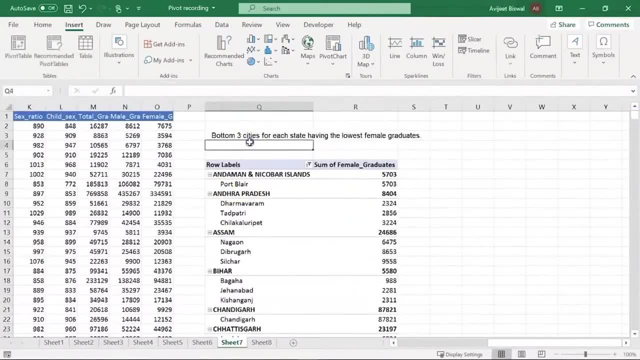 then here we saw how to find out the bottom three cities for each state having lowest female graduates. one thing marked that some of the states did not have three cities. for example, andaman had only one city, that was sport player, but the others we found out the bottom. 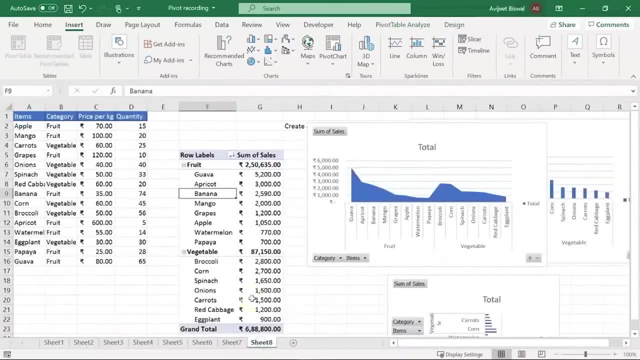 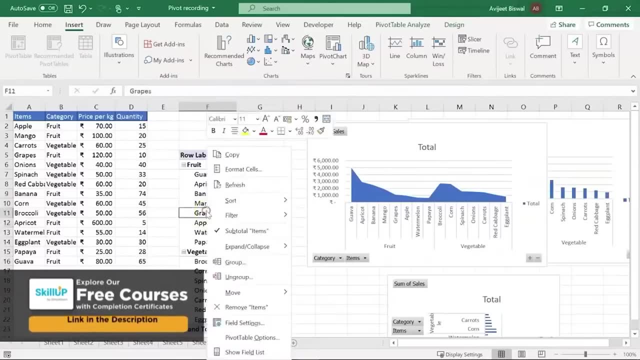 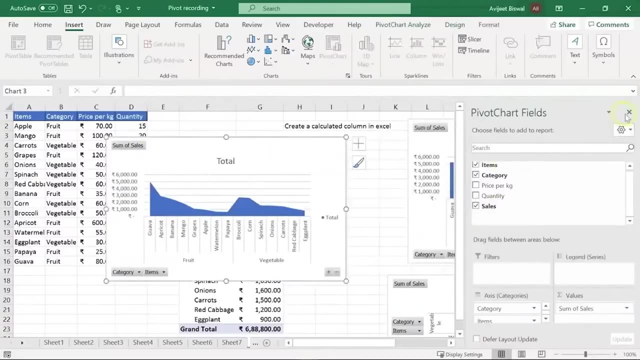 three cities that had the lowest female graduates. finally, we looked at how to create a calculated field in a pivot table. so we saw how to create a calculated field called sales, and then we explored how to create different charts and graphs. so this was an area chart that we saw. 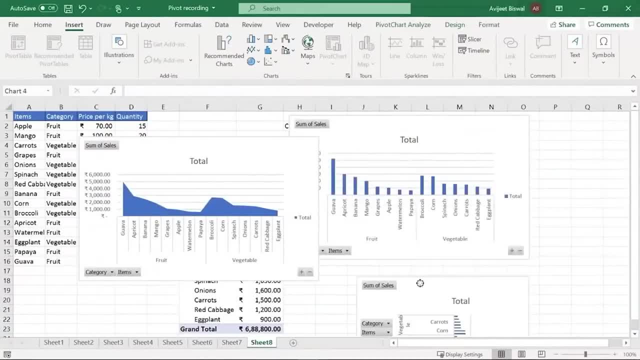 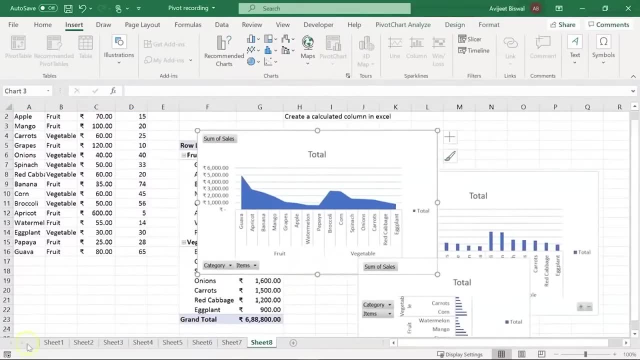 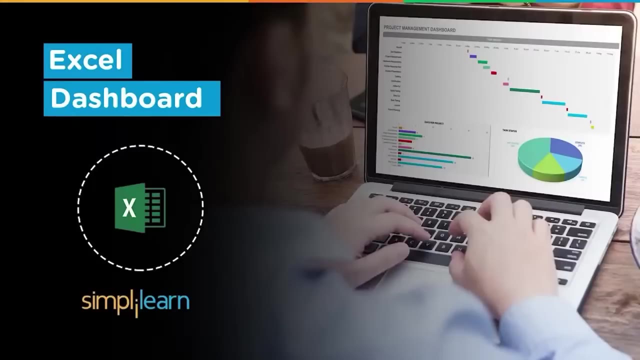 column chart. we also saw, or looked at, a bar chart. that was a horizontal bar chart. similarly, we saw how to create a pie chart as well. in this video we'll be creating two dashboards using a sample sales data set. so if you want to get the data and the 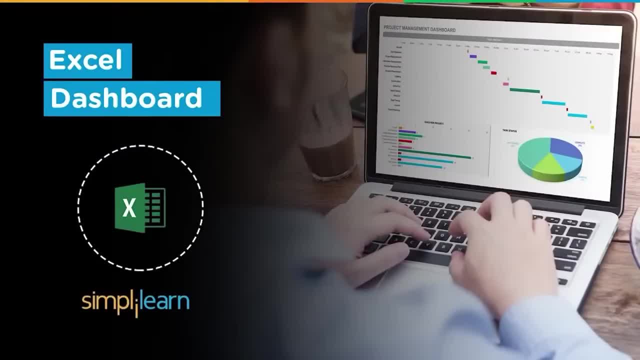 dashboard file that we'll be creating in this demo. then please put your email ids in the comment section of the video. our team will share the files via email. now let's begin by understanding what is a dashboard in excel. a dashboard is a visual interface that provides 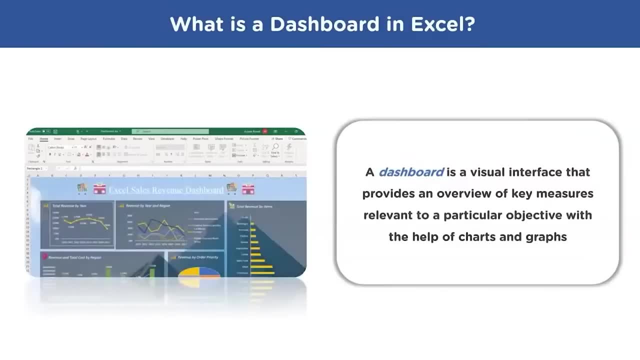 an overview of key measures relevant to a particular objective with the help of charts and graphs dashboards. dashboard reports allow managers to get a high level overview of the business and help them make quick decisions. there are different types of dashboards, such as strategic dashboards, analytical dashboards and operational. 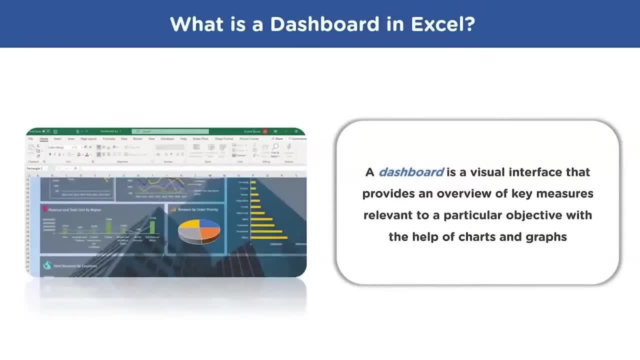 dashboards. an advantage of dashboards is the quick detection of outliers and correlations with comprehensive data visualization. it is time saving as compared to running multiple reports. with this understanding, let's jump into our demo for creating our dashboards. we'll be using a sample sales data set. 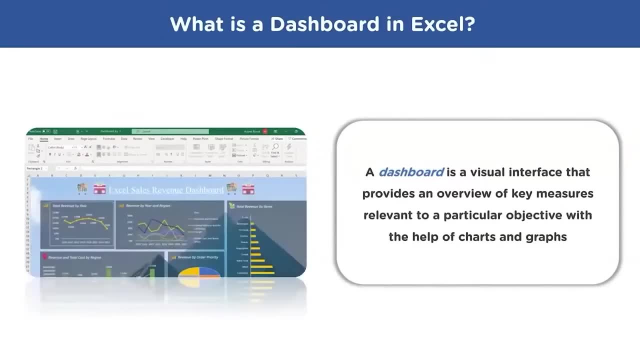 analytical dashboards and operational dashboards. an advantage of dashboards is the quick detection of outliers and correlations with comprehensive data visual visualization. it is time saving as compared to running multiple reports. with this understanding, let's jump into our demo for creating our dashboards. we will be using a sample sales dataset. 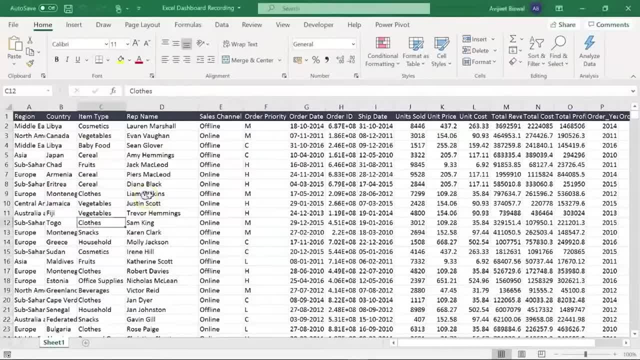 let me show you the dataset first. so here is the sales dataset that we will be using for our demo. so this dataset was actually generated using a simulator and is completely random. it was not validated, though. we have applied certain transformations to the data using power query features. 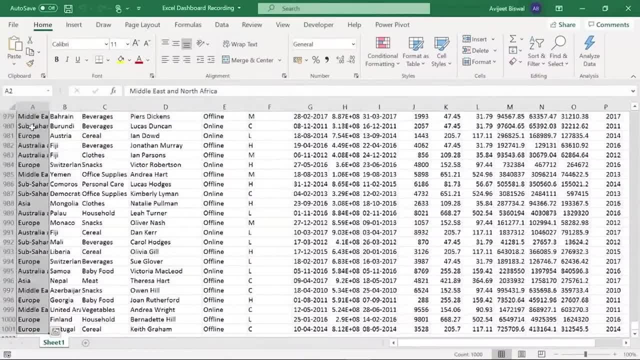 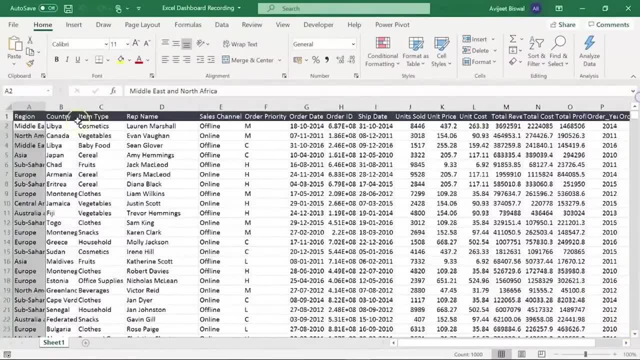 so this data, as you can see, has 1000 rows. so, using the simulator, we had generated 1000 rows of data. similarly, if i go on top, you can see this dataset has 17 columns. now let me give you a brief about each of the columns. 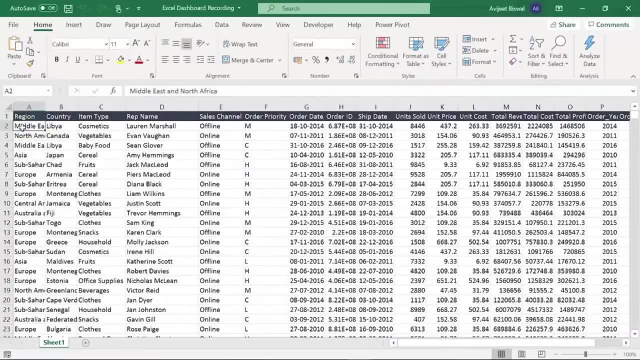 so first we have the region column, so we have middle east and north africa. there is north america, asia, sub saharan africa and others. similarly, we have the country names from which the item was ordered. the third column is the item type, so we have different items: cosmetics, vegetables. 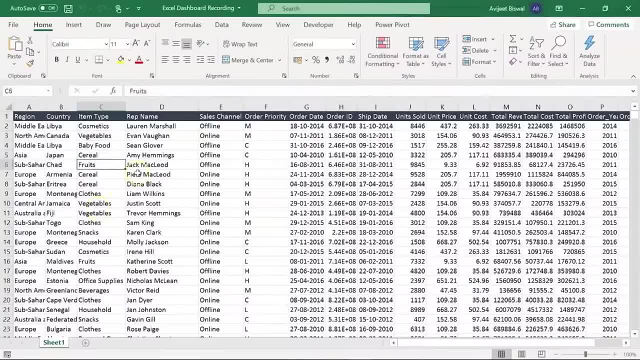 there is baby food, cereal, fruits, etc. then we have the representatives name or you can say this as the customer name who ordered the product. then we have a sales channel column. so there are basically two channels, whether the item was sold offline or online. next we have the order. 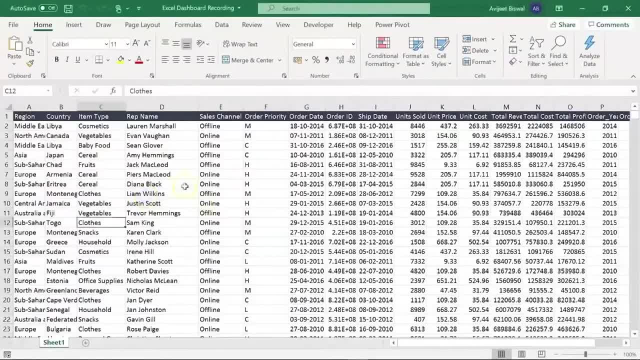 let me show you the data set first. so here is the sales data set that we'll be using for our demo. so this data set was actually generated using a simulator and is completely random. it was not validated, though. we have applied certain transformations to the data using power query features. 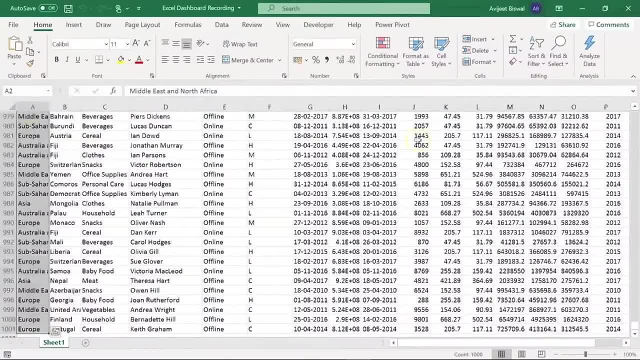 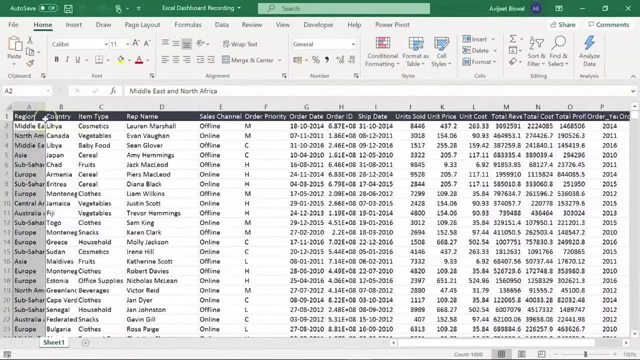 so this data, as you can see, has thousand rows. so using the simulator, we had generated thousand rows of data. similarly, if I go on top, you can see this data set has seventeen columns. now let me give you a brief about each of the columns. so first we have the region column. 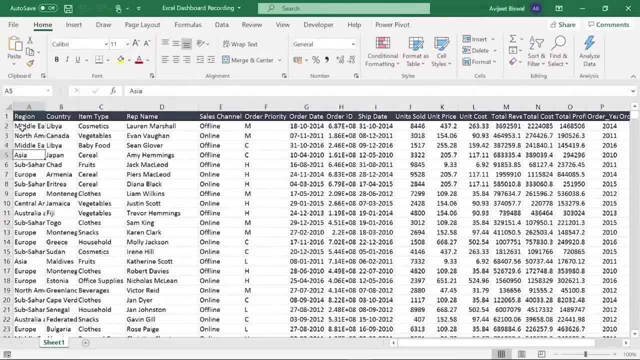 so we have middle east and north africa, there is north america, asia, sub saharan africa and others. similarly, we have the country names from which the item was ordered. the third column is the item type, so we have different items: cosmetics, vegetables, there is baby food, cereal, fruits. 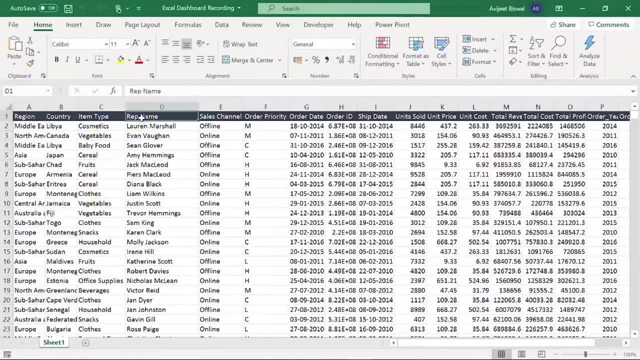 etc. then we have the representatives name or you can say this as the customer name who ordered the product. then we have a sales channel column. so there are basically two channels, whether the item was sold offline or online. next we have the order priority column. now here C. 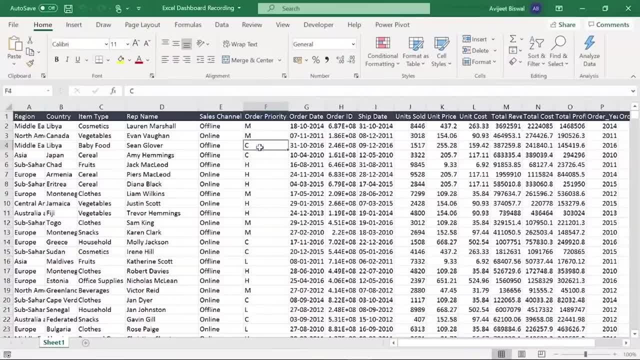 priority column. now here c stands for critical. then we have h, which is for high priority orders, then we have m for medium priority orders and finally we have l, which is for low priority orders. you can see the order date column. then we have the order id, the ship date. 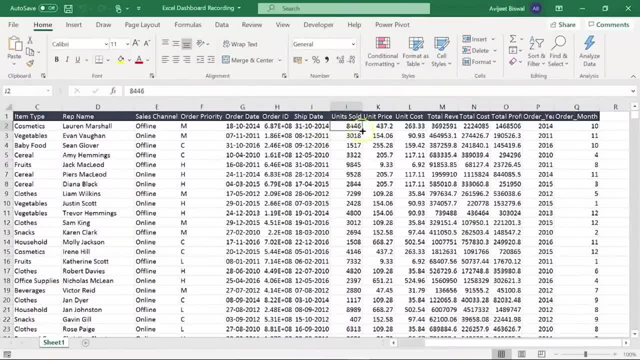 next, we have units sold, which is basically the total number of units sold for each item. then we have the unit price column. this is the price at which each product was sold. then we have the unit cost column, which is basically the production cost for each of the items. 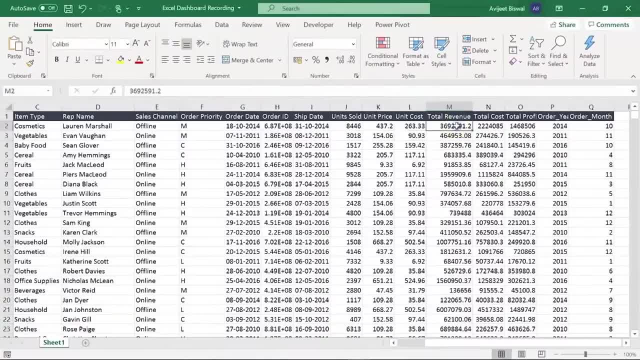 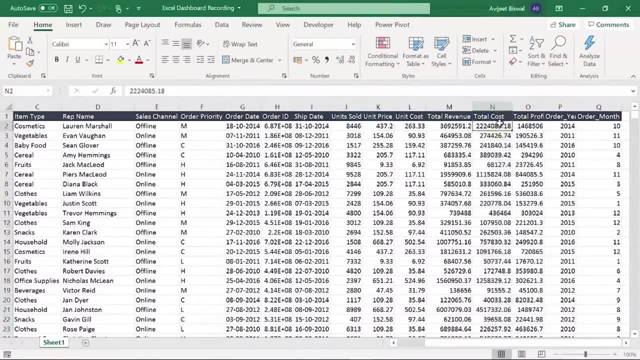 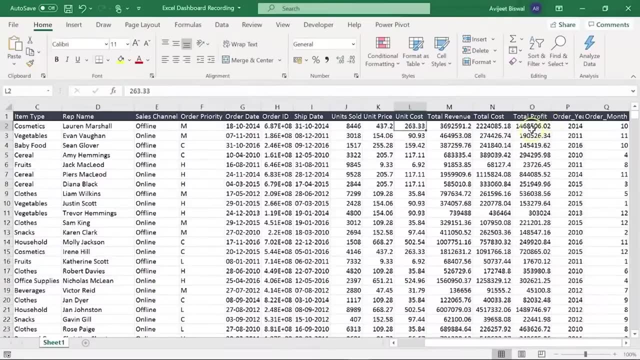 next we have the total revenue. the total revenue is actually the product of units sold and unit price. then we have the total cost column. now, the total cost column is actually the product of units sold and the unit cost. similarly, we have the total profit column, so total profit is the 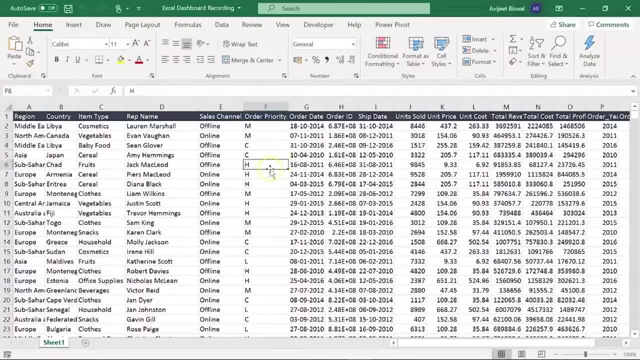 stands for critical. then we have H, which is for high priority orders, then we have M for medium priority orders and finally we have L, which is for low priority orders. you can see the order date column. then we have the order id, the ship date. next we have 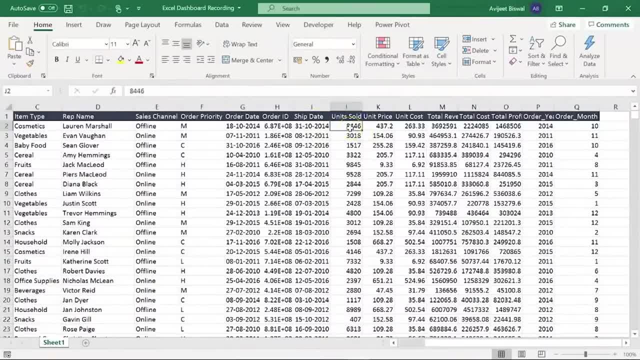 units sold, which is basically the total number of units sold for each item. then we have the unit price column. this is the price at which each product was sold. then we have the unit cost column, which is basically the production cost for each of the items. next we have the total revenue. 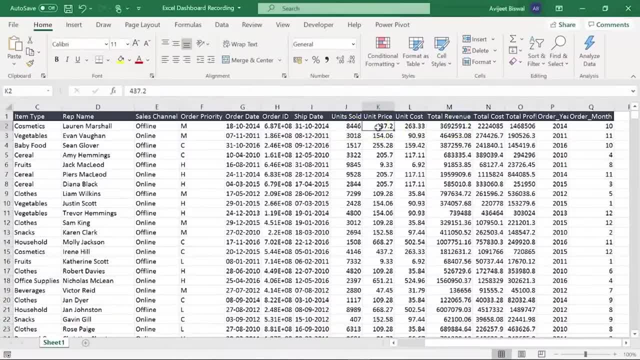 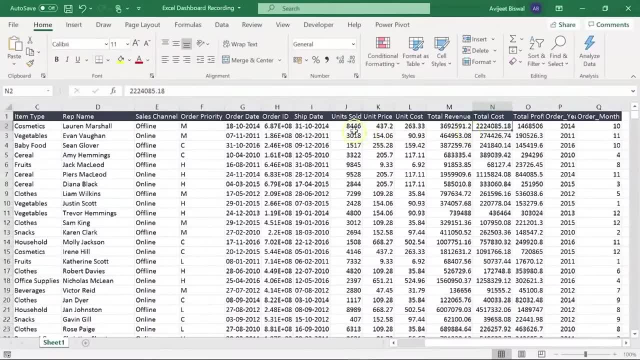 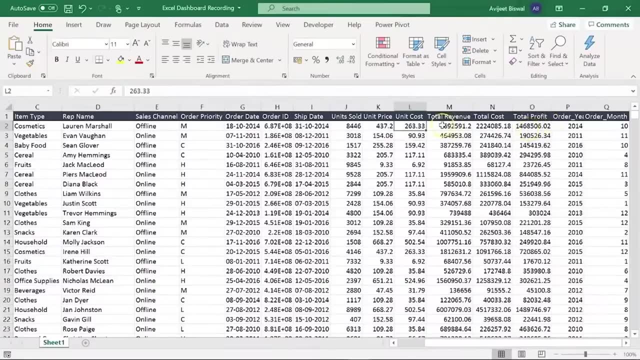 the total revenue is actually the product of units sold and unit price. then we have the total cost column. now, the total cost column is actually the product of units sold and the unit cost. similarly, we have the total profit column. so total profit is the difference between total revenue and the total cost. 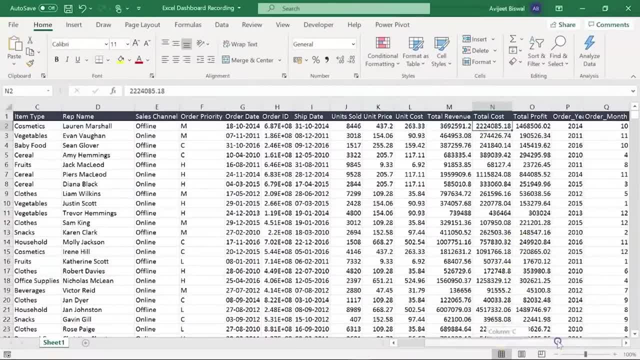 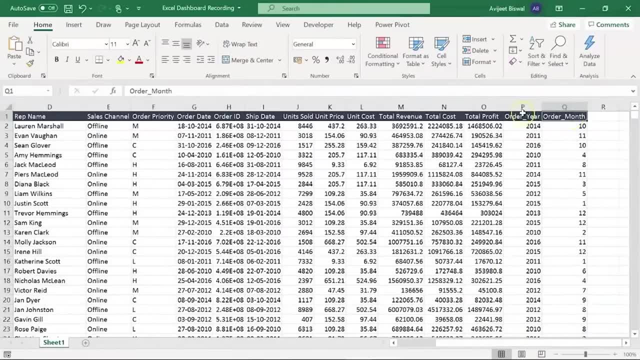 between total revenue and the total cost and finally, we have created two more columns: that is order year and then we have order month. now these two columns were actually generated using the power query features, so we use the order date column, which is this column, and extracted order year and order month. so 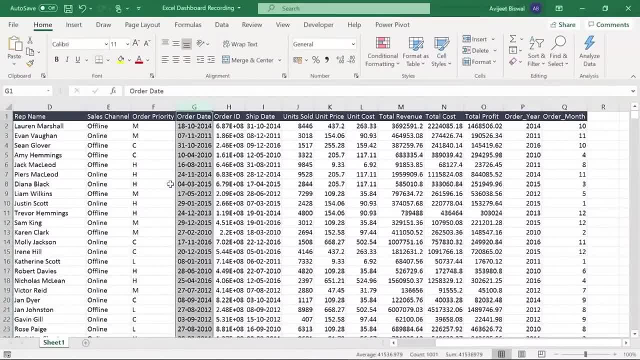 first, we are going to create a revenue dashboard where we will focus on generating reports for revenue by order year, revenue by year and region, revenue by order priority and much more. we'll create separate pivot tables and pivot charts and format them to make them look more interesting and presentable. we'll 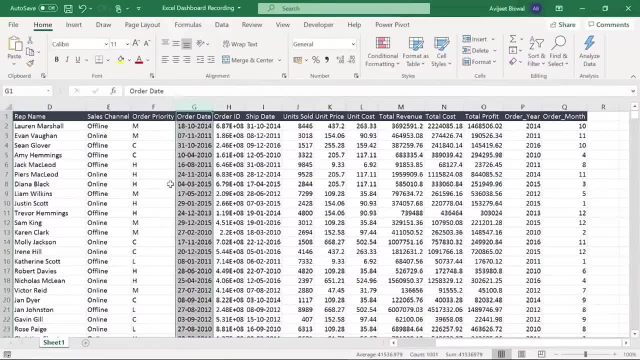 add slices and timeline to our dashboards in order to filter it based on specific fields. now let's create our first report to see the total revenue generated each year. so we need to create a pivot table for this. I'll click on a cell in my data set. 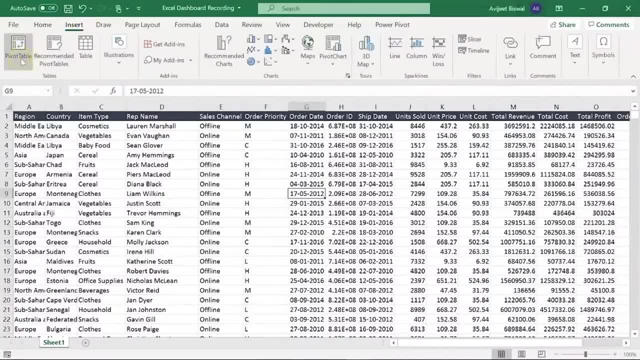 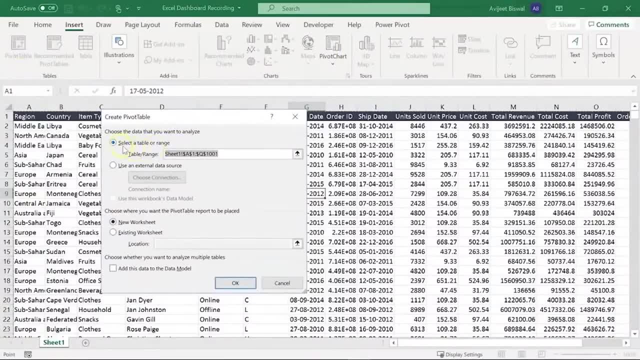 and then I'll go to the insert tab. here we have the option to select the pivot table. I click on this. you can see my table range is selected. next I want to place my pivot table in a new worksheet and let's just click on OK, there you go. 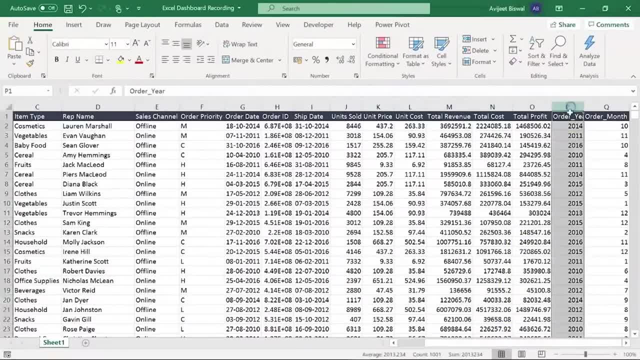 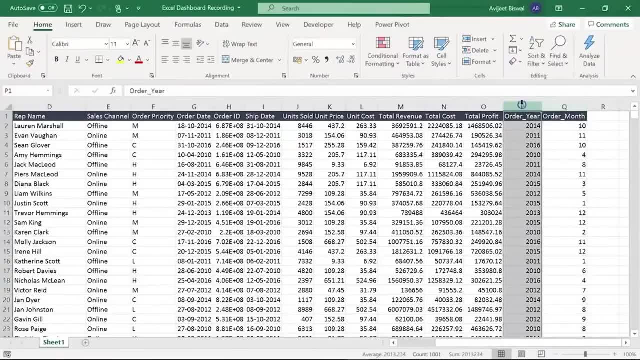 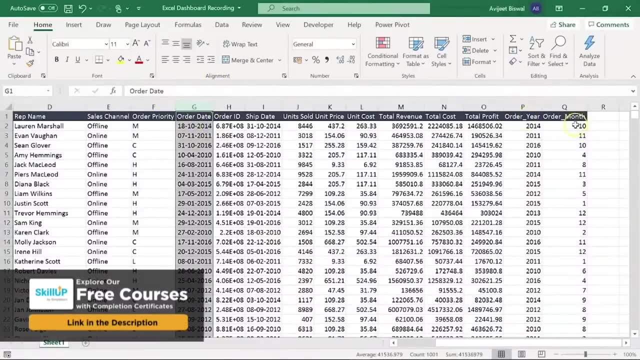 and finally, we have created two more columns. that is order year and then we have order month. now these two columns were actually generated using the power query features, so we used the order date column, which is this column, and extracted order year and order month. so first we are going to create a revenue dashboard. 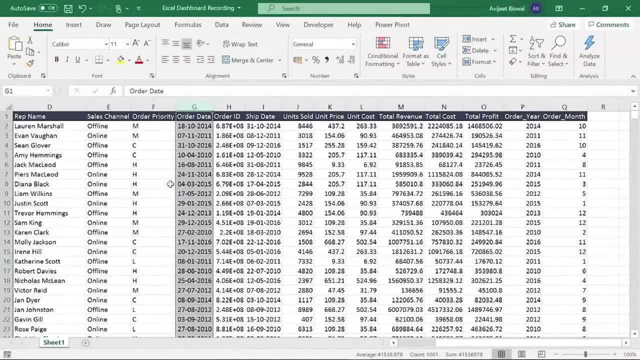 where we will focus on generating reports for revenue by order year, revenue by year and region, revenue by order priority and much more. we will create separate pivot tables and pivot charts and format them to make them look more interesting and presentable. we will add slices and timeline to our dashboards in order to 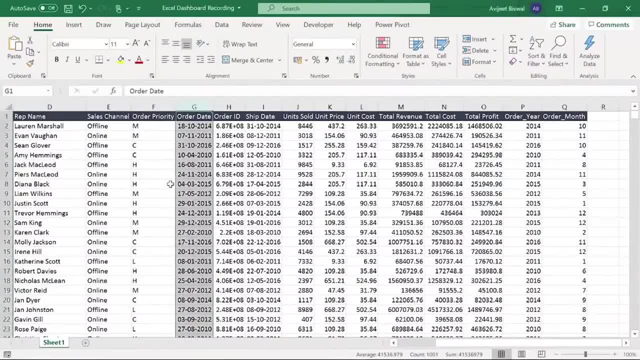 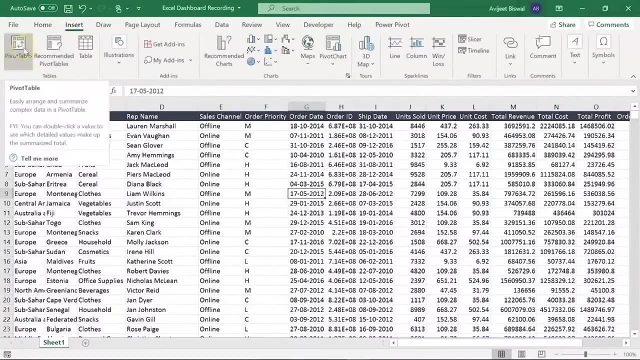 filter it based on specific fields. now let's create our first report to see the total revenue generated each year. so we need to create a pivot table for this. i will click on a cell in my data set and then i will go to the insert tab. here we have the option to select. 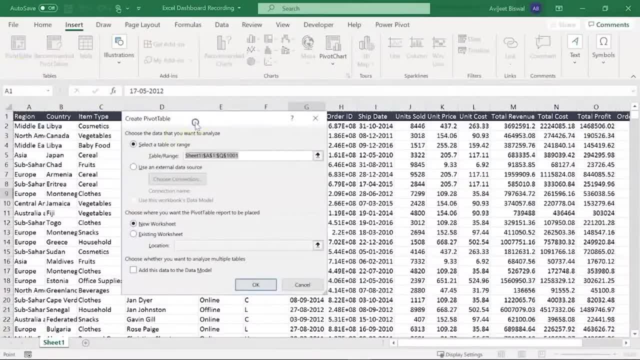 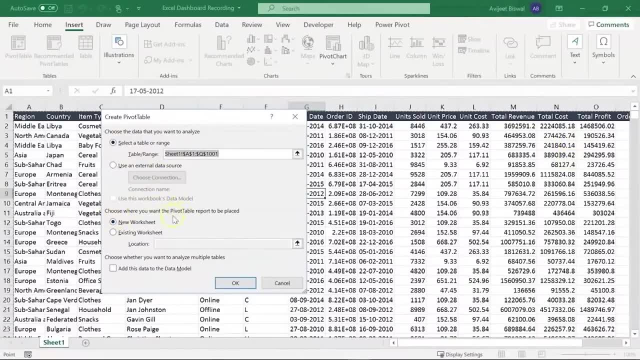 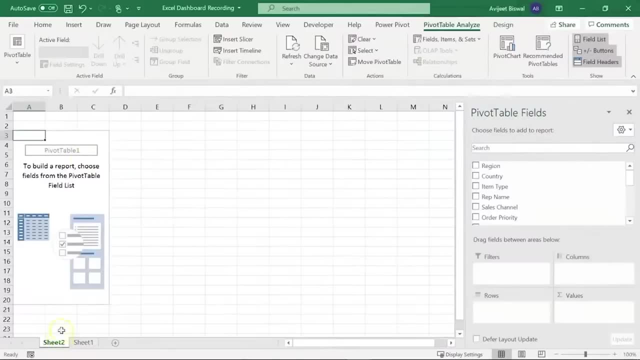 the pivot table. i click on this. you can see my table range is selected. next, i want to place my pivot table in a new worksheet and let's just click on. ok, there you go. so we have a new sheet where i can place my pivot table. so first, 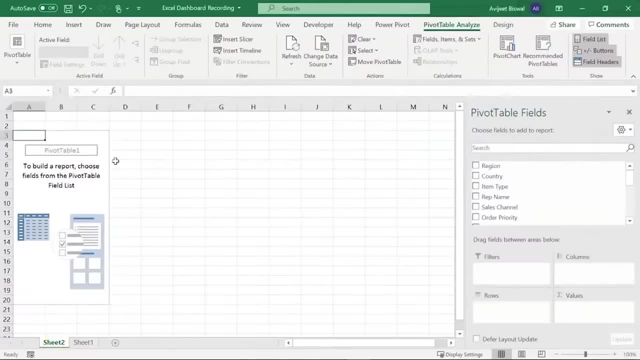 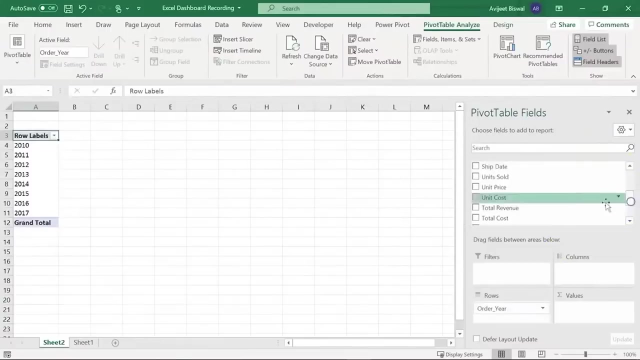 so we have a new sheet where I can place my pivot table. so first I need to find the total revenue generated by each year. so what I'll do is and drag my order year column under rows and then I'll select the total revenue column under values. you can see, I have my pivot chart ready now. if you want, you can sort. 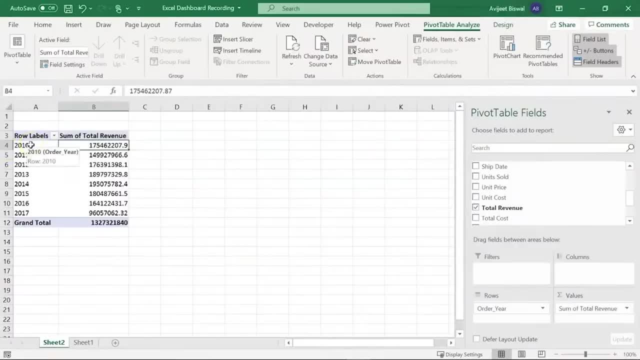 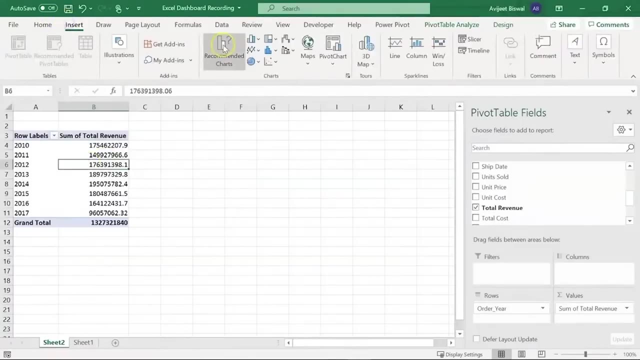 this. so from the data you can see, we have order year from 2010 to 2017. now, based on this data, let's create on our Pivot Chartväg chart. so i'll click on any cell, go to insert and here you have the option to select recommended. 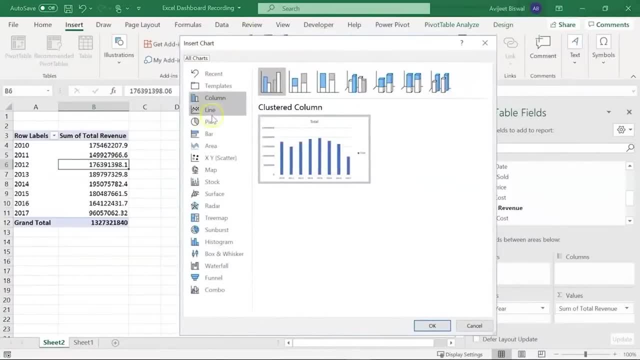 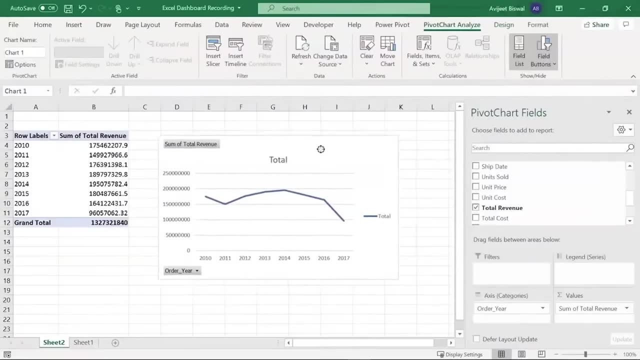 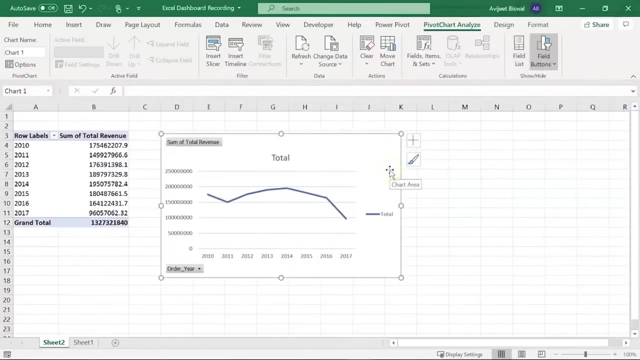 charts. i click on this now. actually i want a line chart, so i'll click on line here and select. ok, there you go. so we have successfully created our first pivot chart. now let me show you how you can format this chart to make it more readable. so first let me delete these, so i'll right click and 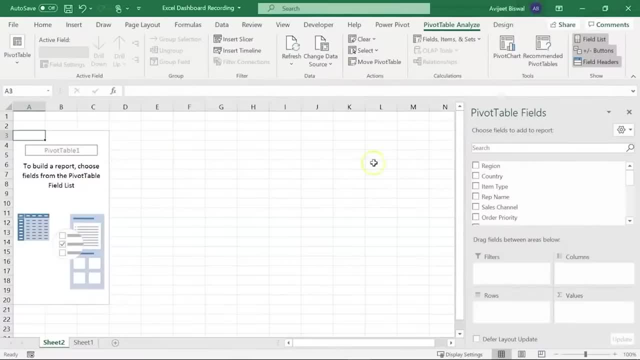 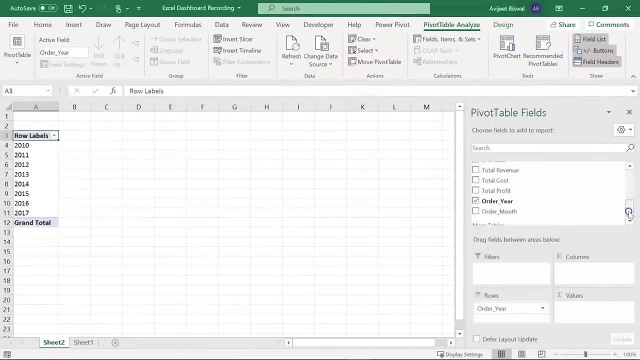 i need to find the total revenue generated by each year. so what i will do is i will drag my order year column under rows and then i will select the total revenue column under values. you can see, i have my pivot chart ready now. if you want, you can sort this. 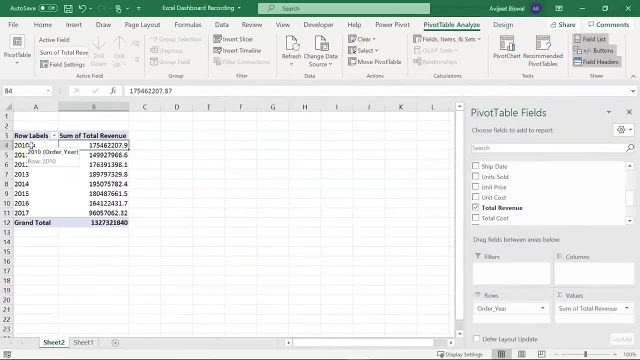 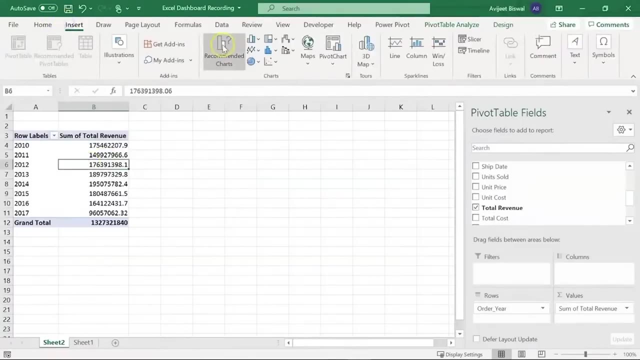 so from the data you can see, we have order year from 2010 to 2017. now, based on this data, let's create our pivot chart. so i will click on any cell, go to insert, and here you have the option to select recommended charts. i click on this. 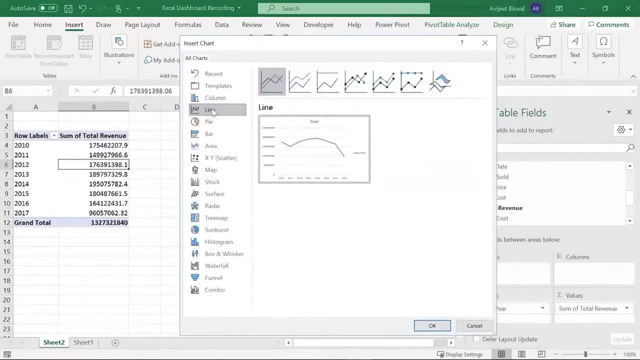 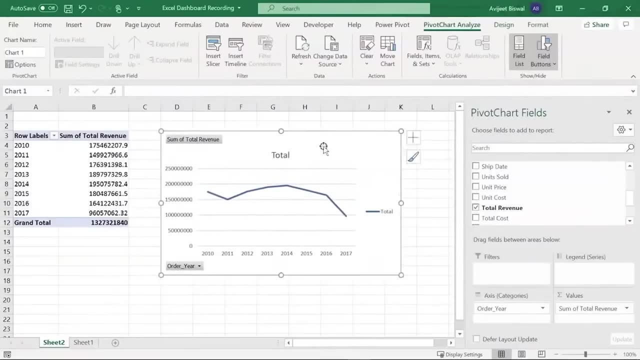 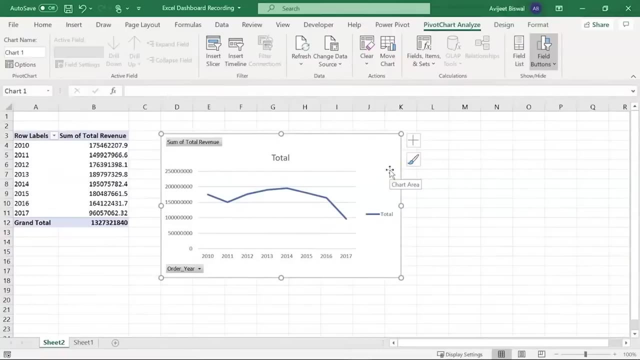 now. actually, i want a line chart, so i will click on line here and select. ok, there you go. so we have successfully created our first pivot chart. now let me show you how you can format this chart to make it more readable. so first let me delete these. 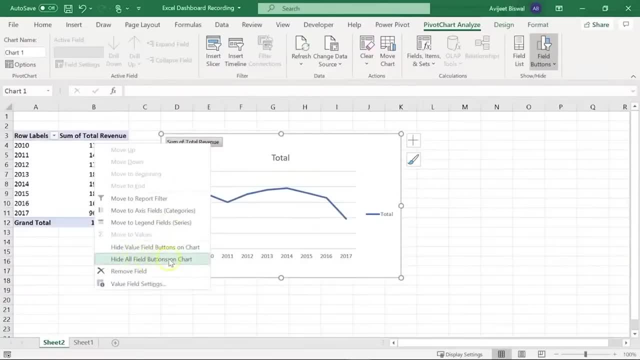 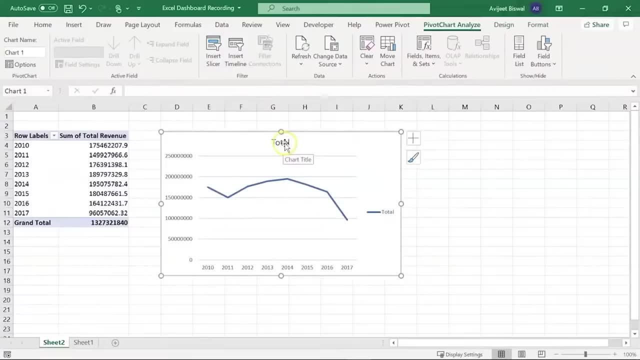 so i will right click and select hide all field buttons on the chart. so this will delete the buttons present on the chart. now let me go ahead and edit the chart title. so the title i want is total revenue. i will type it down by year, alright, next. 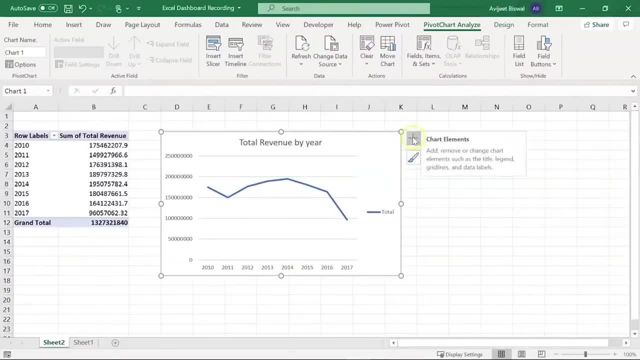 let's do a few more transformations. so if i click on this plus sign, which is actually for chart elements, we have some options like to add axis, axis titles, chart title, data labels, this grid, lines, legend and others. ok, so let's remove the legend. now you can see the total legend. 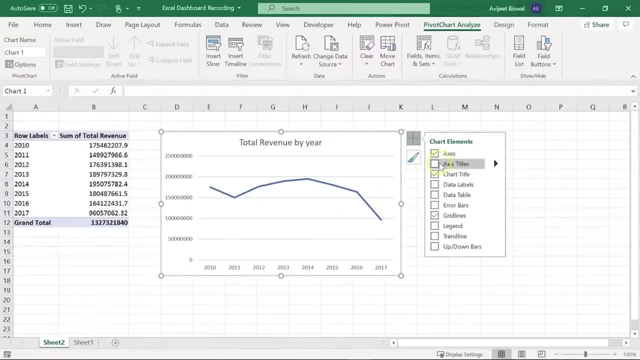 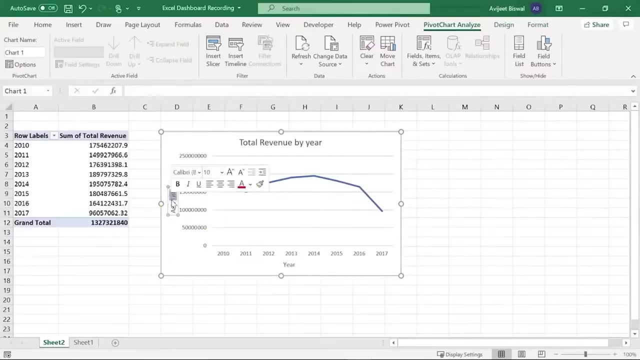 is gone. now let me add axis titles. so we label our x axis and y axis. so here under x axis i can write it as year. similarly, on the y axis i will put revenue. ok, now you can move a bit. alright, now let me select this chart. 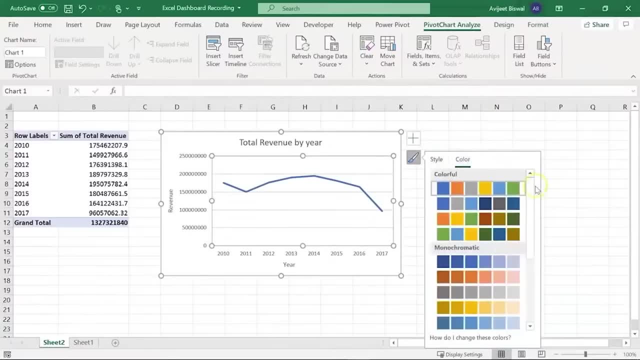 style option and go to colors first. here i will select yellow color. ok, then let me go back to style. let's select a new style from this list. i want this style. ok, now you can also add data labels. so i will just click on data labels. you can see we have. 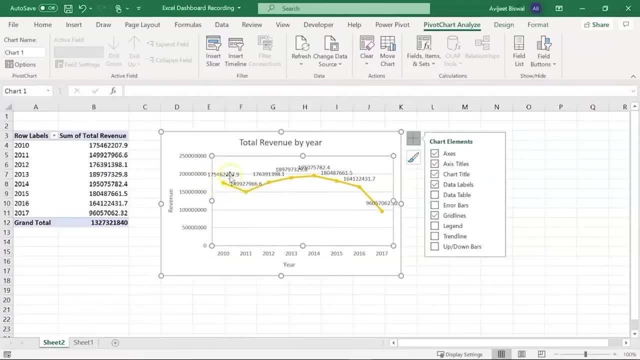 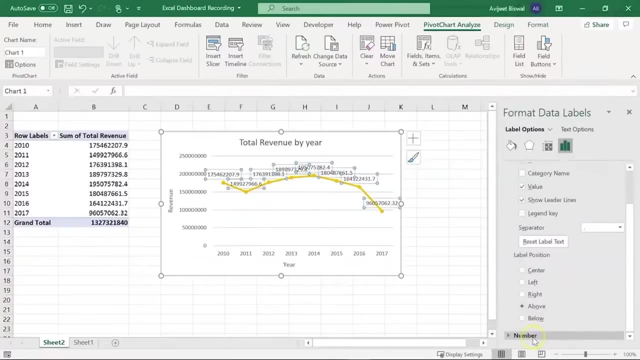 the revenue for each of the years. now this is not readable at all, so we will format this a bit. if i click on this arrow here, i have more options. if i scroll down, you can see we have something called as number. here i will expand this and. 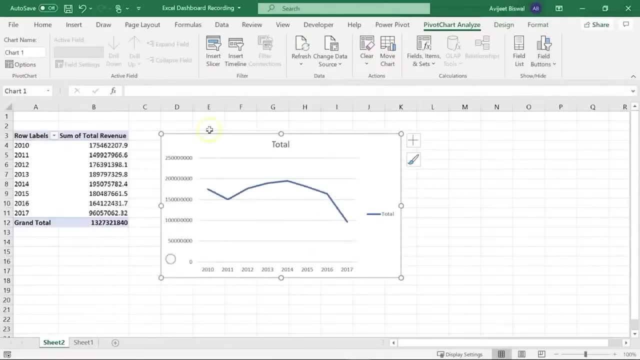 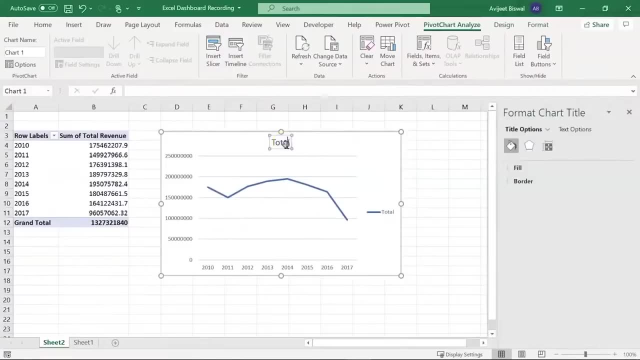 select hide all field buttons on the chart. so this will delete the buttons present on the chart. now let me go ahead and edit the chart title. so the title i want is total revenue. i'll type it down by year, all right. next let's do a few more transformations. so if i click on this plus sign, 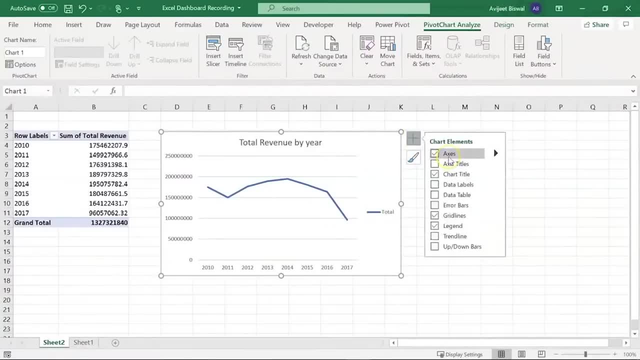 which is actually for chart elements. we have some options, like to add access, access titles, chart title, data labels, this grid lines, legend and others. okay, so let's remove the legend. now you can see the total legend is gone. now let me add access titles. so we'll label our x-axis and y-axis. so here under x-axis, i can write it as: 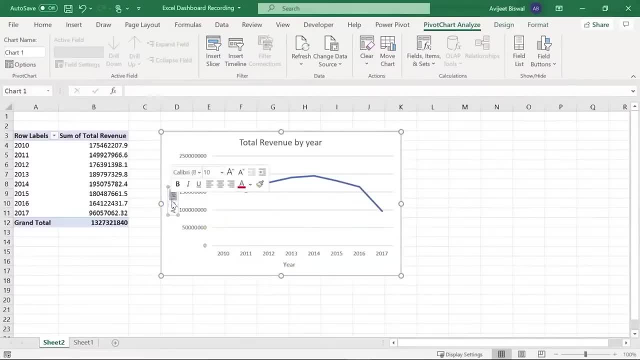 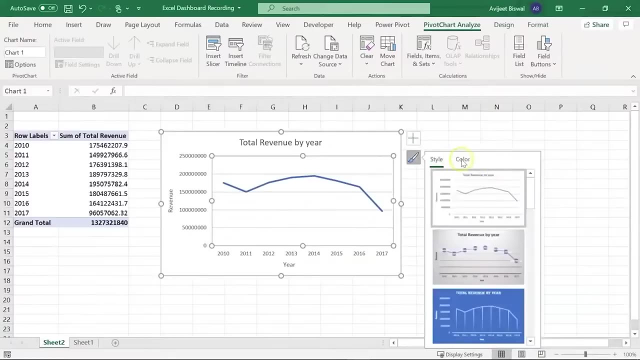 year. similarly on the y-axis, i'll put revenue. okay, now you can move a bit. all right, now let me select this chart style option and go to colors. first here i'll select yellow color, okay, and then let me go back to style. let's select a new style from. 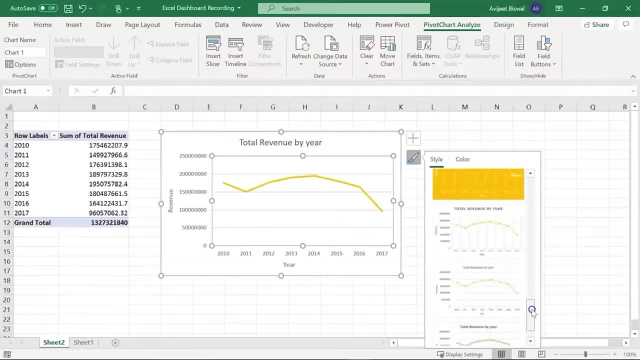 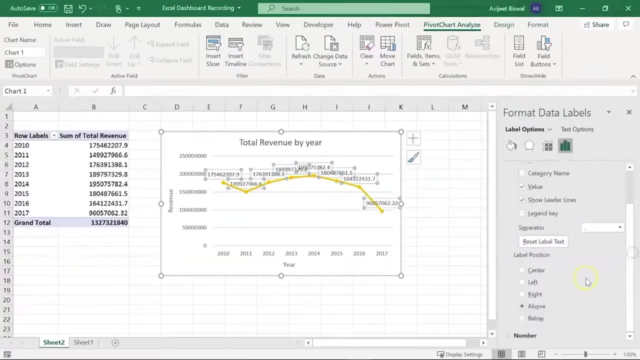 this list. i want this style. okay, now you can also add data labels. so i'll just click on data labels. you can see we have the revenue for each of the years. now this is not readable at all, so we'll format this a bit. if i click on this arrow here, i have more options. if i scroll down, you can see we have. 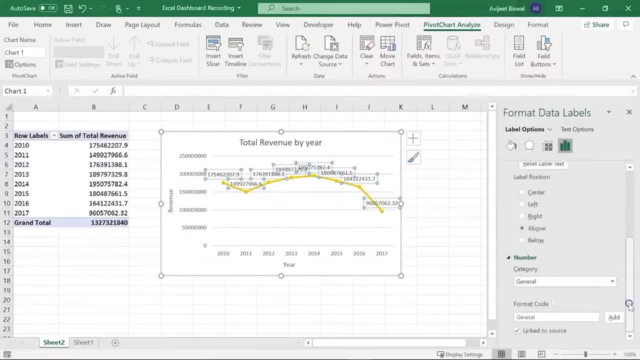 something called as number. here i'll expand this and under category i'll select custom. now, here we'll give a format code which is a bit different. so this is actually a kind of a formula. so i'll write: if my revenue value is greater than, let's say, 9 lakhs 99 000. 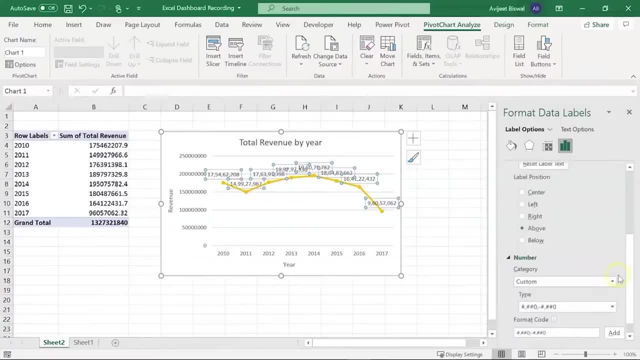 under category, i will select custom. now here we will give a format code which is a bit different. so this is actually a kind of a formula. so i will write if my revenue value is greater than, let's say, 9 lakhs 99 thousand. let me make sure. 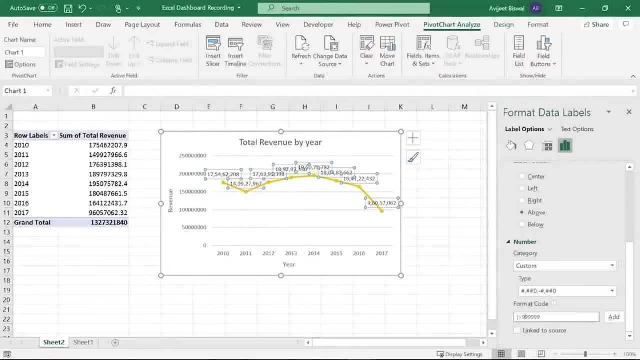 there are six, nines here, so one, two, three, four, five and six. ok, we are good to go. i will close the bracket. i will give a hash, give two commas. so if the revenue is greater than 9 lakhs 99 thousand, i will put it in the format of millions. 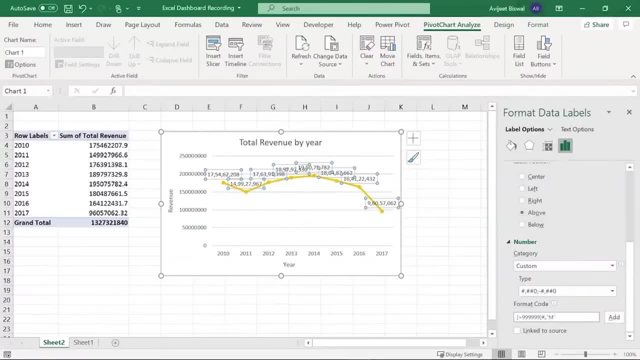 so, within double quotes, i will write m, i will give a semi colon, followed by another hash, and if the value is less than the desired number, it should be zero million. let me click on add. alright, you can see how nicely we have formatted our data and you see, here we have. 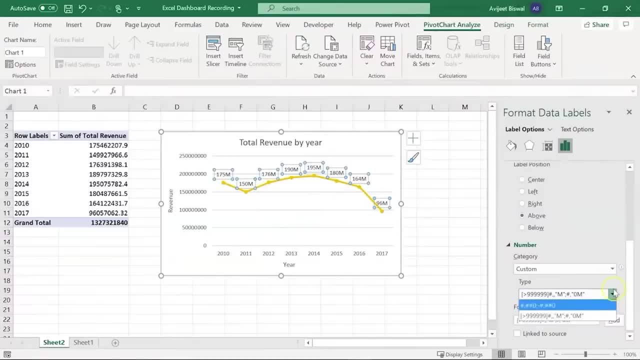 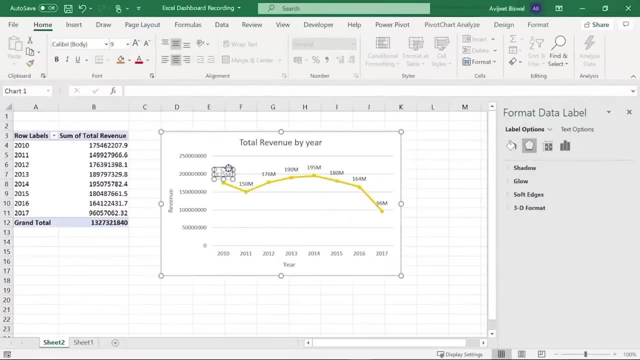 added the new format, which is in millions. alright, now, if you want, you can go ahead and adjust the boxes. let me move this a bit up. i will delete this now. if you notice this line chart, you can make a few conclusions. for example, if you see here in: 2010, the total revenue generated was nearly 175 million. now this came down to 150 million in 2011. then the revenue constantly grew. from 2011 till 2014 it reached 195 million, and after 2014 it again came down to. 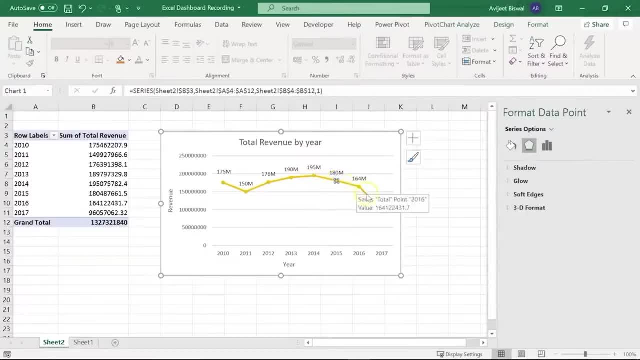 180 million, and the revenue dropped significantly between 2016 and 2017. in 2017, the revenue was just 96 million. now, before moving ahead to my next chart, let me just rename this sheet, so i will write it as revenue by year. alright, 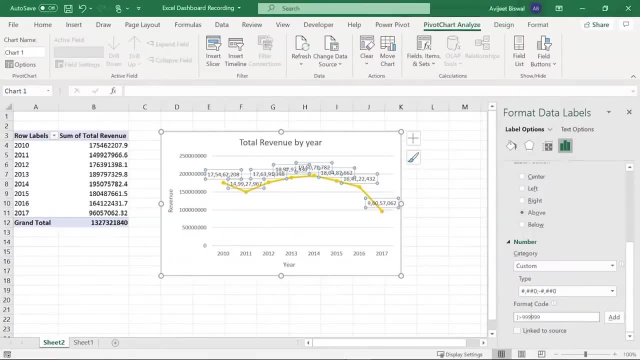 let me make sure there are six, nines here, so one, two, three, four, five and six. okay, we are good to go. i'll close the bracket, i'll give a hash, give two commas. so if the revenue is greater than 9 lakhs 99 000, i'll put it in the format of. 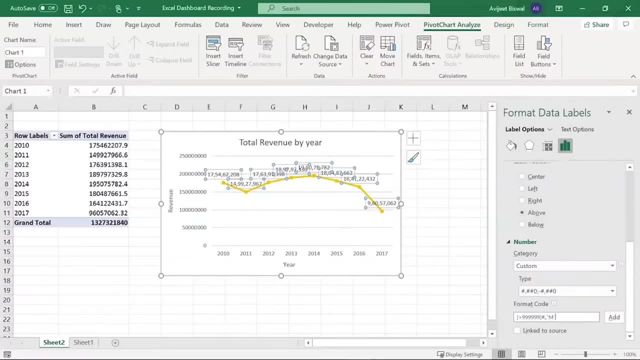 millions. so within double quotes i'll write m, i'll give a semicolon followed by another hash, and if the value is less than the desired number, it should be 0 million. let me click on add. all right, you can see how nicely we have formatted our data. 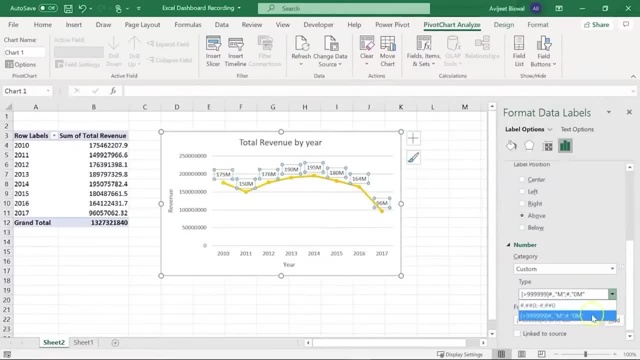 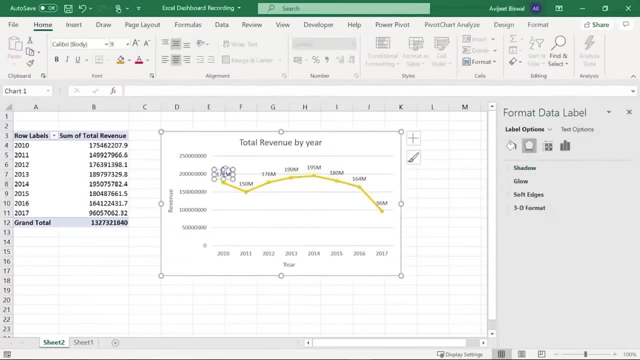 and you see, here we have added the new format, which is in millions. all right now, if you want, you can go ahead and adjust the boxes. let me move this a bit up. i'll delete this now. if you notice this line chart, you can make a few conclusions. for example: 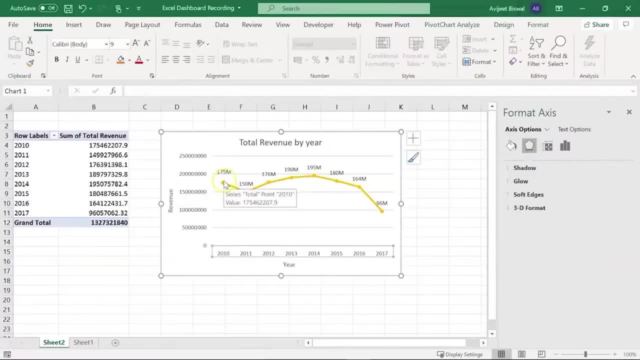 if you see here, in 2010 the total revenue generated was nearly 175 million. now this came down to 150 million. in 2011, then the revenue constantly grew. from 2011 till 2014 it reached 195 million and after 2014 it again came down to 180 million and the revenue dropped. 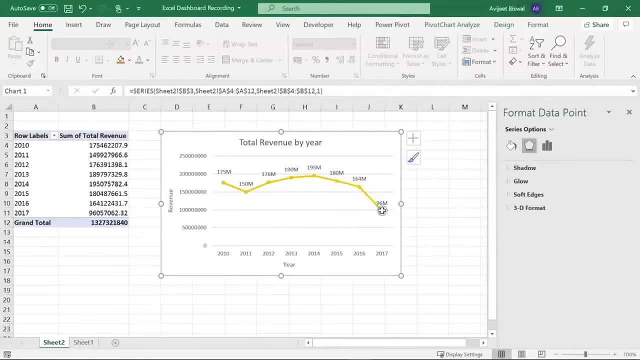 significantly between 2016 and 2017. in 2017, the revenue was just 96 million. now, before moving ahead to my next chart, let me just rename this sheet, so i'll write it as revenue by year. all right, now let's analyze the revenue generated each year in different regions. 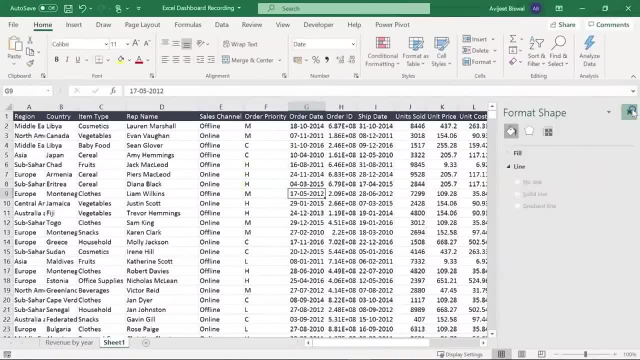 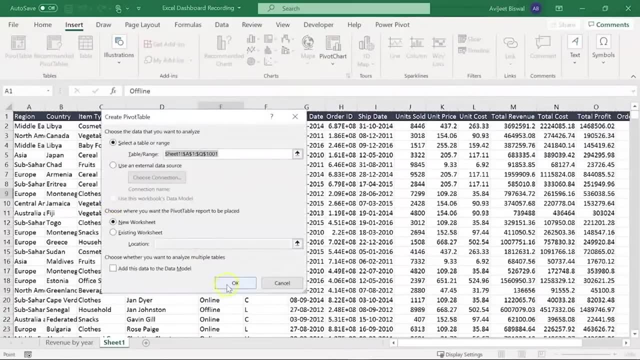 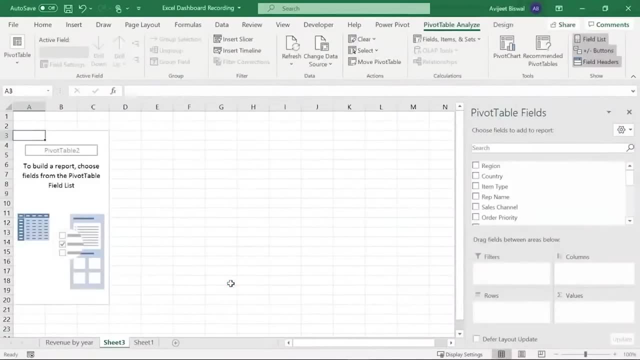 so for this we'll create another pivot table. let me close this. i'll click on any cell, go to insert and select pivot table. i just click ok so that my pivot table is placed on a new sheet. all right now. this time we want the revenue by each year and region, so first of all let's drag. 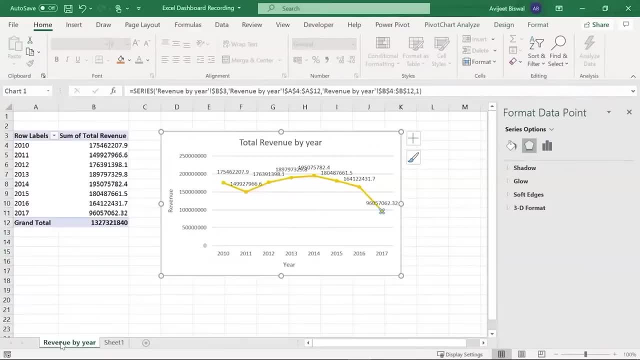 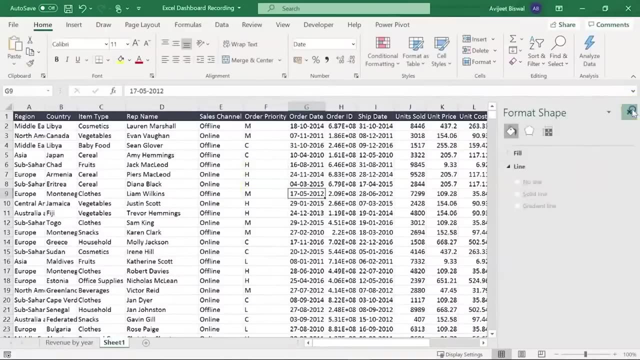 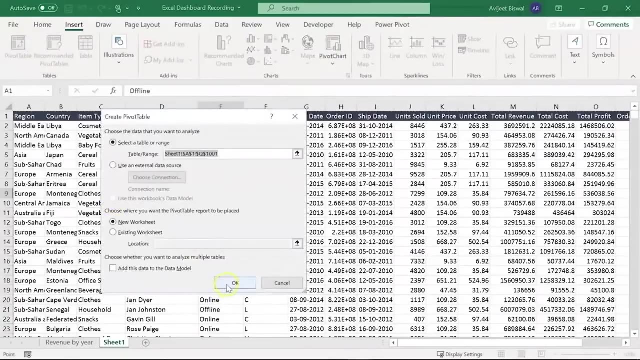 now let's analyze the revenue generated each year in different regions. so for this we will create another pivot table. let me close this. i will click on any cell, go to insert and select pivot table. i will just click ok so that my pivot table is placed on a new sheet. 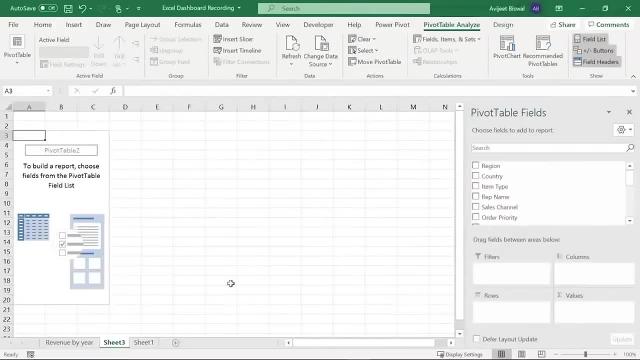 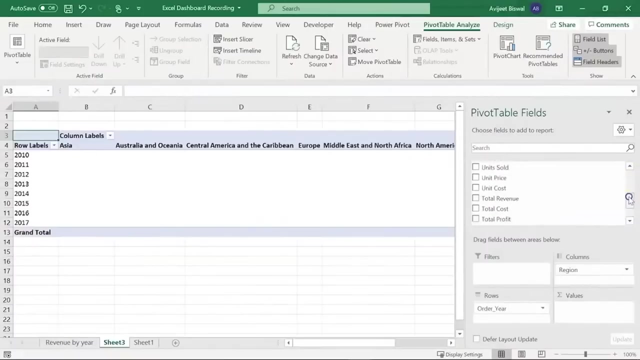 alright, now this time we want the revenue by each year and region. so first of all let's drag region to columns, then let's drag the order year column under rows and then i will select total revenue onto values. so here you can see, we have the pivot. 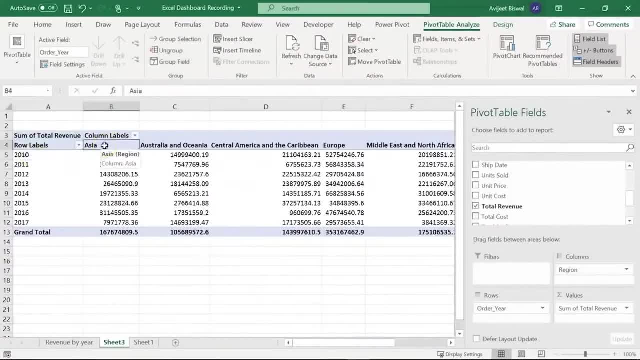 table ready. so for 2010, you can see in each year, this was the revenue generated. similarly, if you see for 2013, this was the total revenue generated in europe and we have for other years as well. now let's create a line chart based on this. 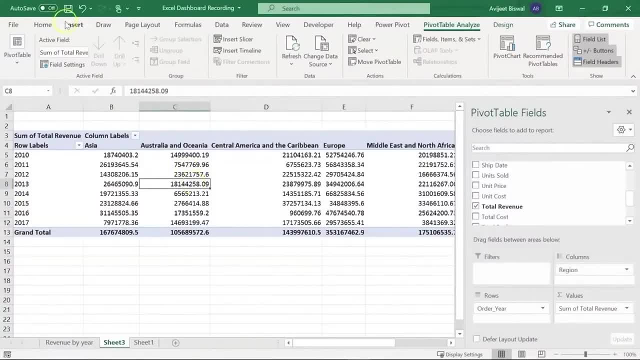 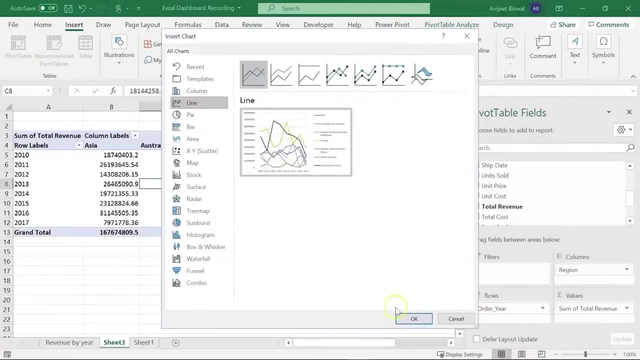 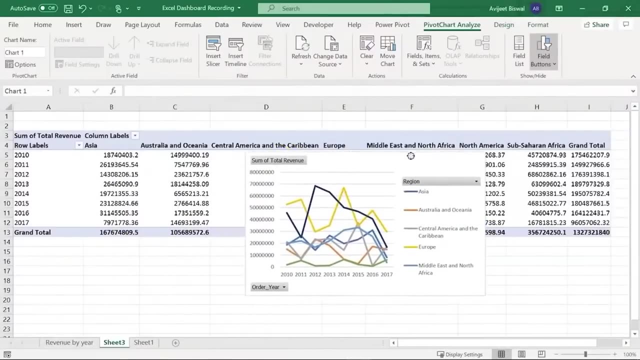 pivot table. so i will select any cell in the pivot table i will go to insert and i will click on recommended charts from this list. i will select my line chart and click on ok, there you go. so we have our next pivot chart ready. so on the right, you see the different regions. 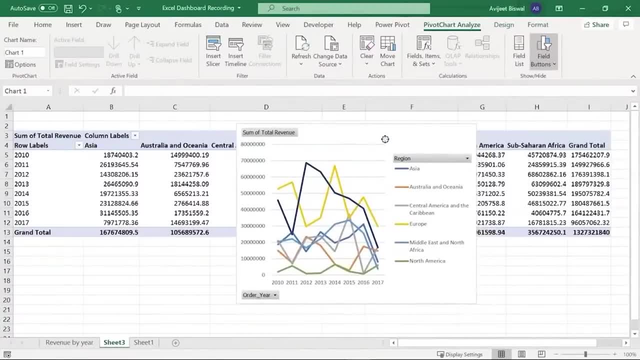 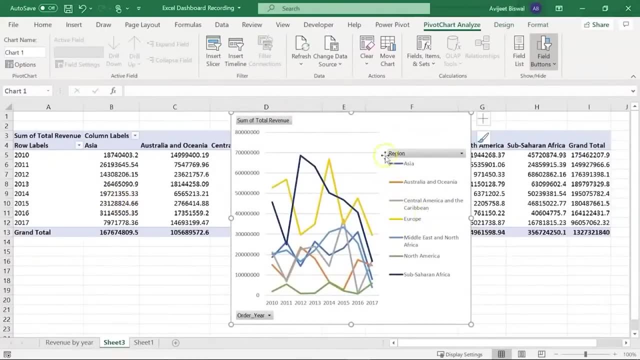 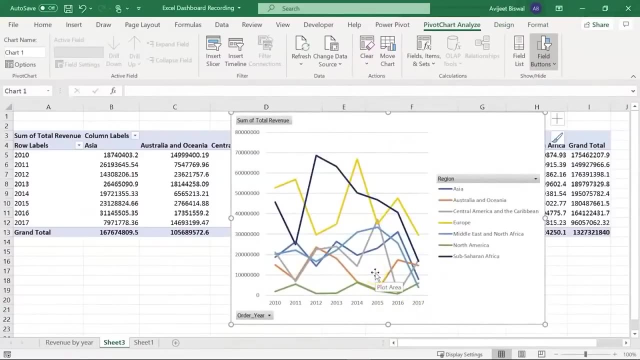 that are present in different colors. let me just expand it so that you can see all the regions we have. so in total, we have 7 regions and each of the regions have been represented in different colors. so if you notice this graph for the sub saharan african. 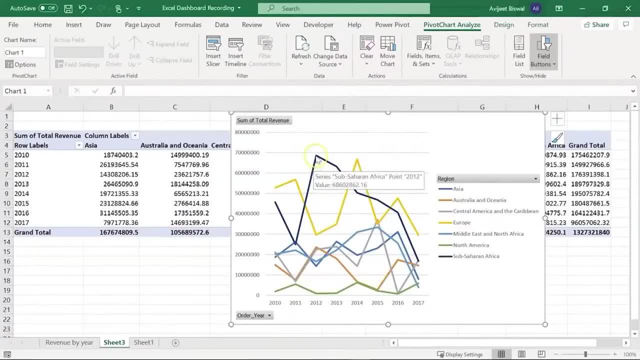 region. in 2012, sub saharan africa made the highest amount of sales. now, from the sample data, you can also tell that the revenue for north america has been significantly low compared to other regions. similarly, if you see, for europe, this was the revenue trend between 2010 and 2017. 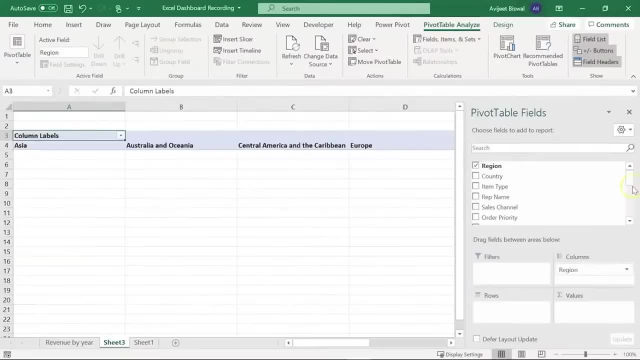 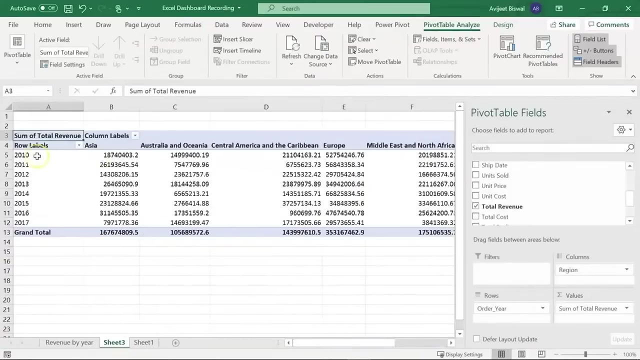 region to columns, then let's drag the order year column under rows and then i'll select total revenue onto values. so here you can see, we have the pivot table ready. so for 2010, you can see, in asia, this was the revenue generated. similarly, if you 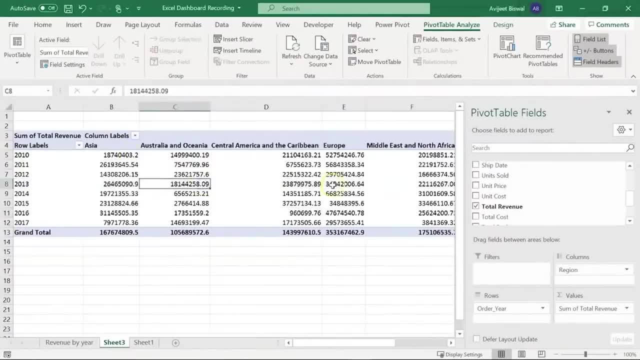 see for 2013. this was the total revenue generated in europe and we have for other years as well. now let's create a line chart based on this pivot table. so i'll select any cell in the pivot table, i'll go to insert and i'll click on. 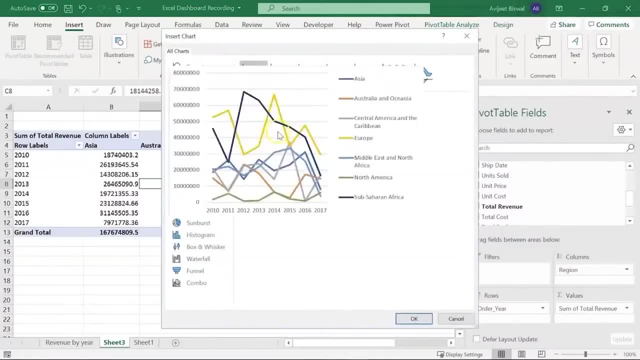 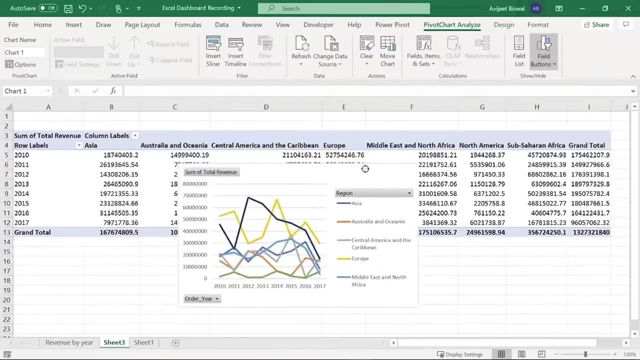 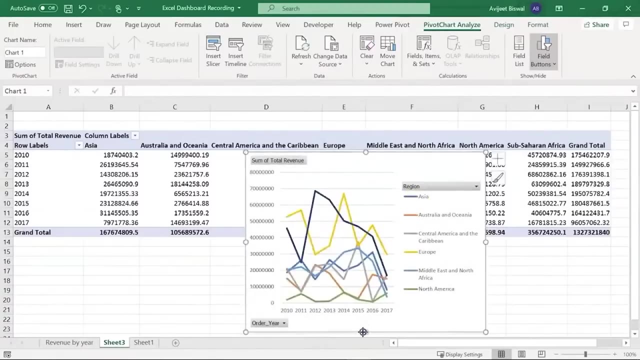 recommended charts. from this list i'll select my line chart and click on ok. there you go. so we have our next pivot chart ready. so on the right, you see the different regions that are present in different colors. let me just expand it so that you can see all the regions we have. so in total, 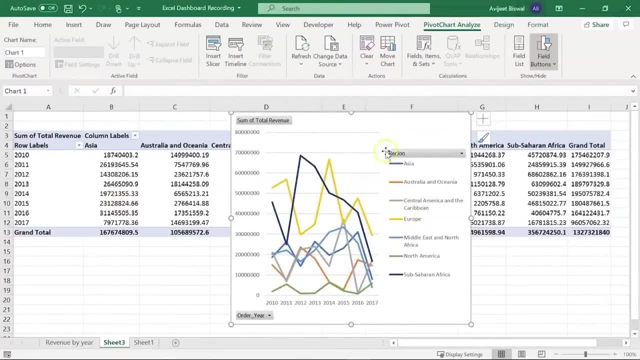 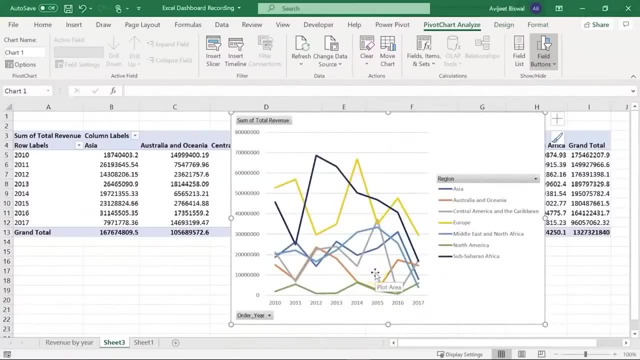 we have seven regions and each of the regions have been represented in different colors. so if you notice this graph for the sub-saharan african region, in 2012, sub-saharan africa made the highest amount of sales. now, from the sample data, you can also tell that the revenue for 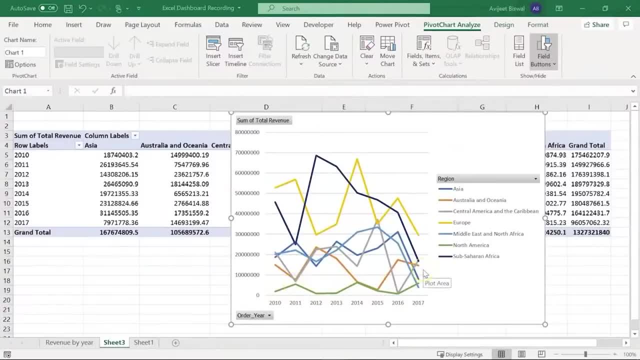 America has been significantly low compared to other regions. similarly, if you see for Europe, this was the revenue trend between 2010 and 2017. so if you see here, in 2011 the sales were at this level, then it significantly dropped in 2012, then in 2013 there was a huge spike and then in again came down in 2015 and 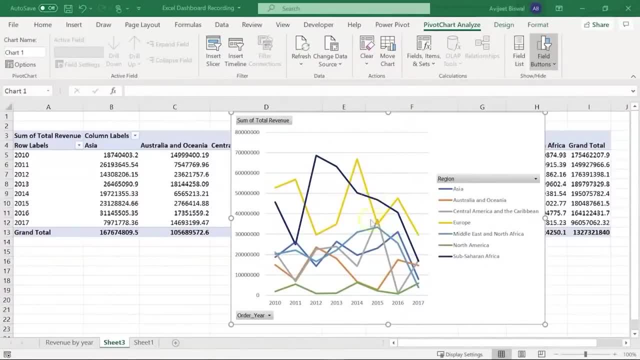 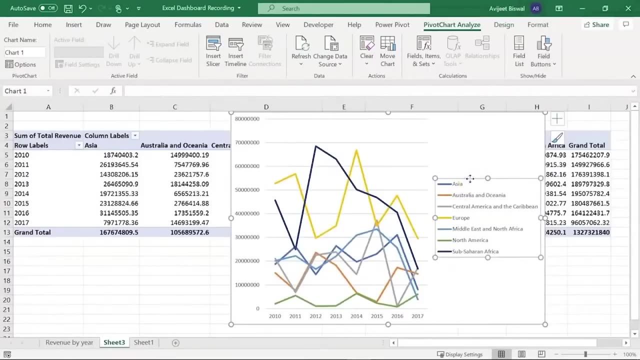 so on. so you can make your own conclusions by looking at these line charts. now let's format this chart. so first of all, let's delete the field buttons present on the chart and we'll also delete the legend. all right now, let me just show you how to delete the legend. all right now, let me just show you how to. 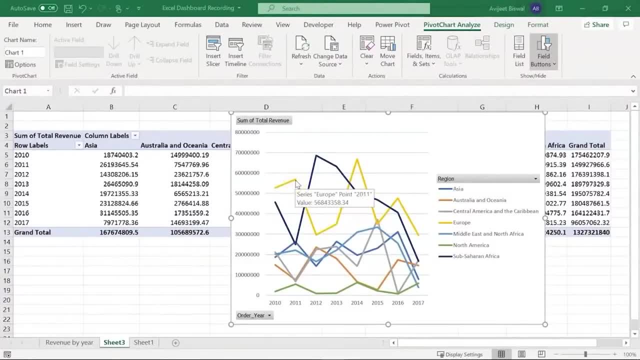 so if you see here, in 2011 the sales were at this level, then it significantly dropped in 2012, then in 2013 there was a huge spike and then in again came down in 2015, and so on. so you can make your own. 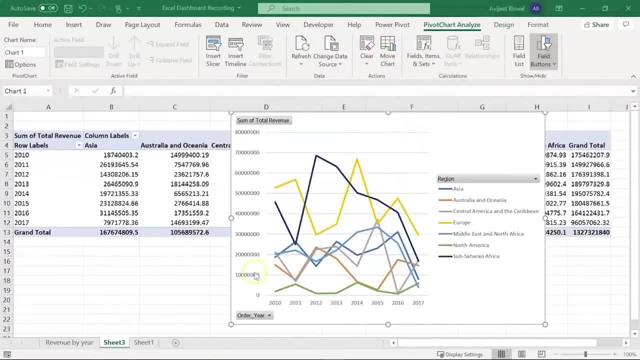 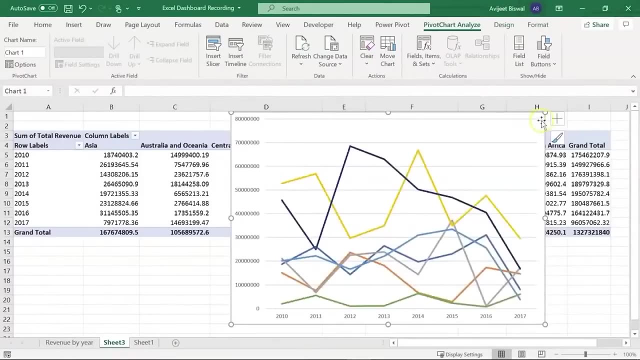 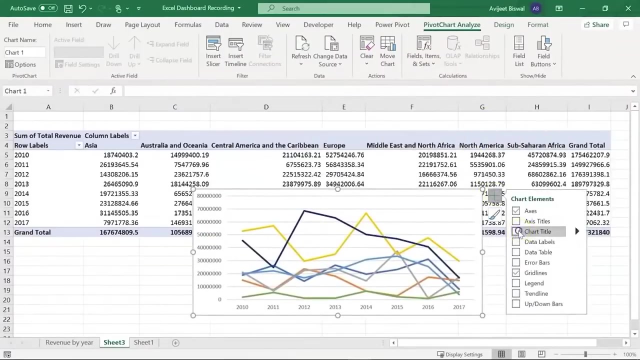 conclusions by looking at these line charts. now let's format this chart. so, first of all, let's delete the field buttons present on the chart and we will also delete the legend. alright, now let me just reduce the size of the chart. next, we will add a chart title. so 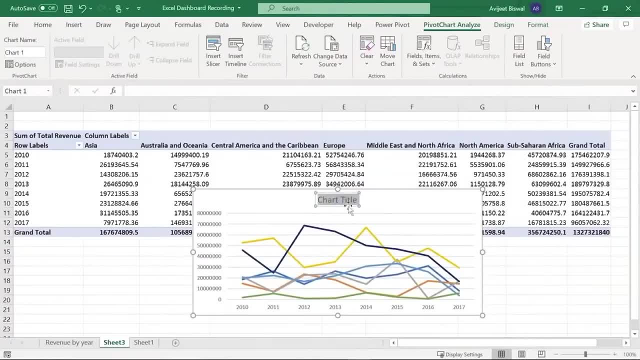 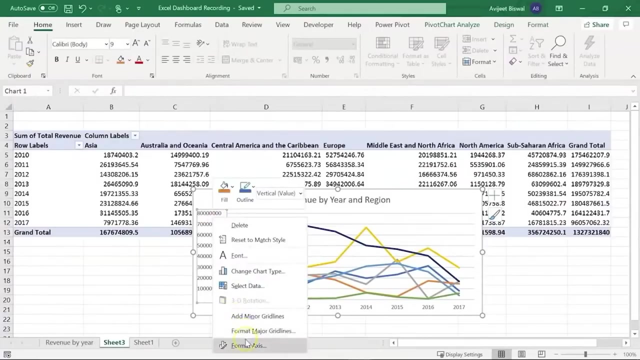 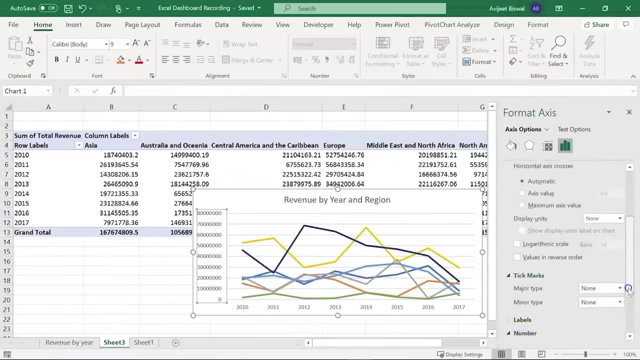 we will give the title as revenue by year and region. ok, you can also format the y axis in terms of millions. so i will right click on this axis and i will select format axis. i will scroll down and here we have the number drop down. let me scroll again. 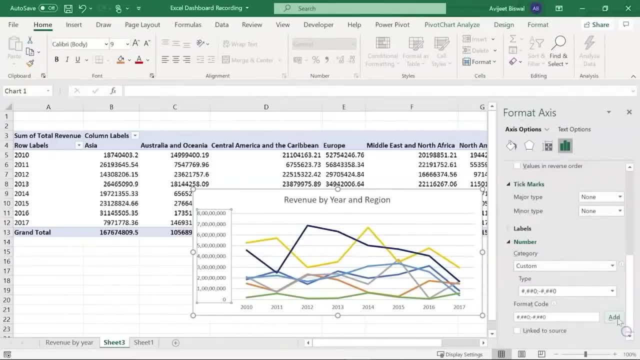 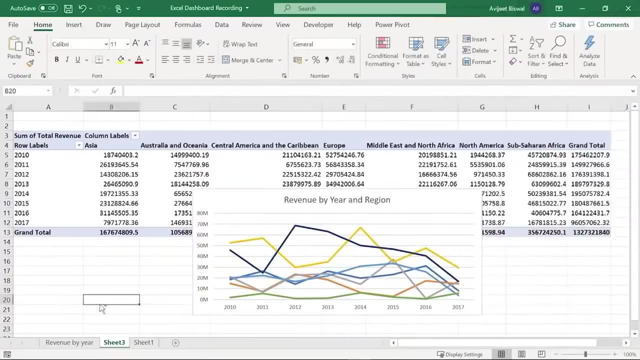 under category, i will select custom and we will use this format that we created for our previous chart. there you go. you can see our axis labels have been changed in terms of millions now, so let's close this and let me save it. now you can reduce the font size or 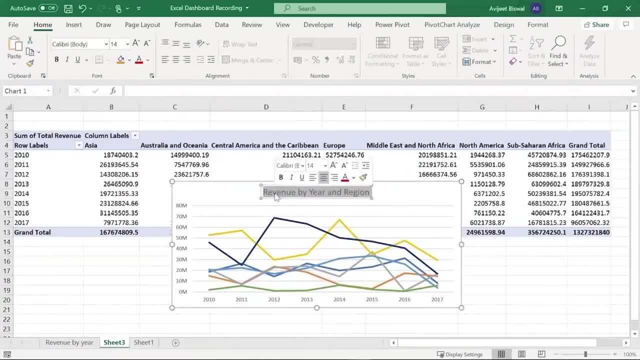 increase the font size. let me just show you. suppose you want to increase the font size of the chart title, so you just select it and from here you can either reduce or you can increase. you can see now it's 12. if you want, you can make it 16. 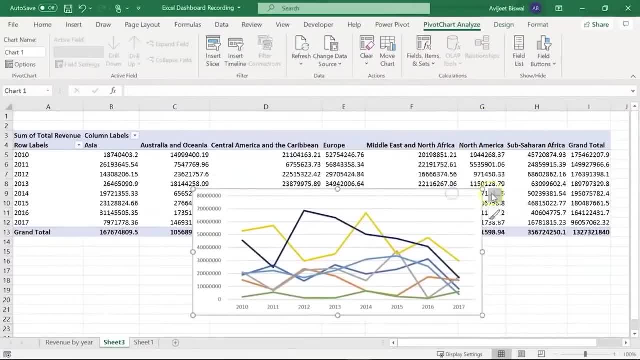 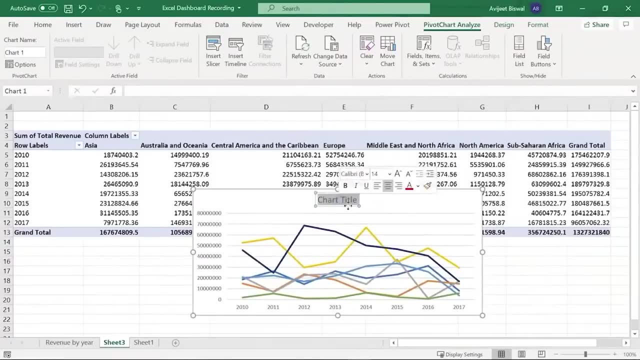 delete the legend. all right, now let me just show you how to reduce the size of the chart. next, we'll add a chart title, so we'll give the title as revenue by year and region. okay, you can also format the y-axis in terms of millions, so I'll right-click on this axis. 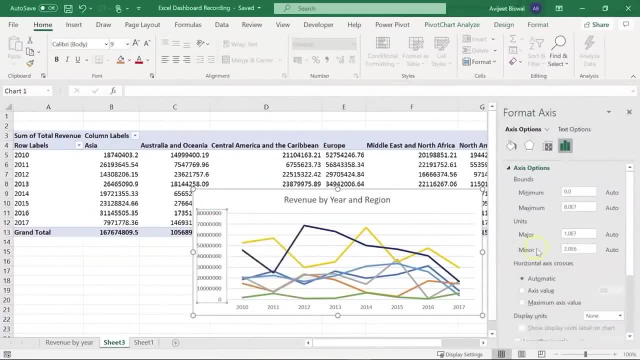 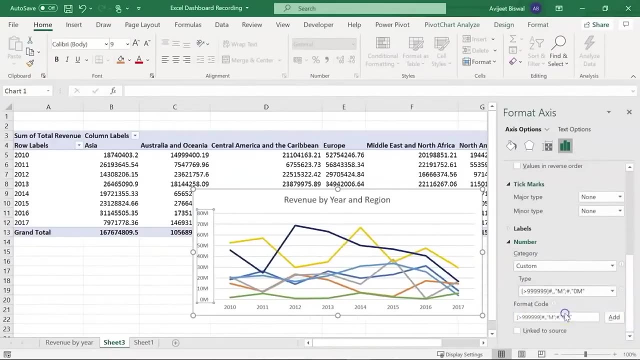 and I'll select format, axis. I'll scroll down and here we have the number drop down. let me scroll again under category. I'll select custom and we'll use this format that we created for our previous chart. there you go. you can see our axis labels have been changed in terms of millions now, so let's close this and let 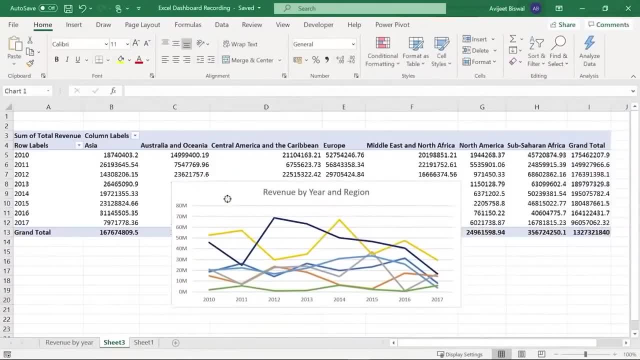 me save it now. you can reduce the font size or increase the font size. let me just show you. suppose you want to increase the font size of the chart title, so you just select it and from here you can either reduce or you can increase. you can see. 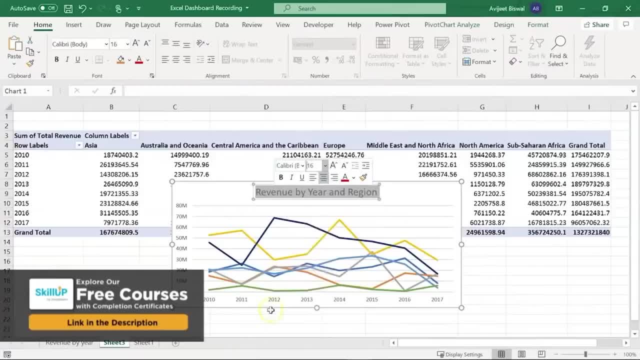 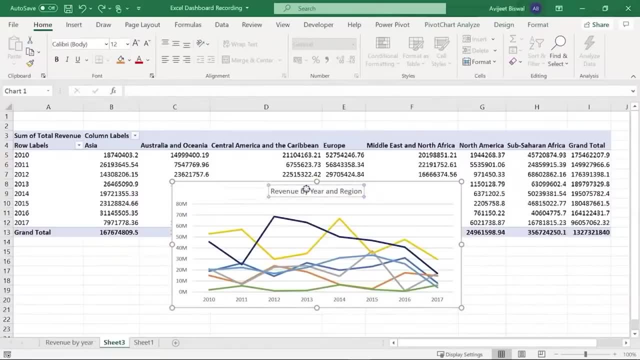 now it's 12. if you want, you can make it 16. similarly, you can also edit the axis labels also by selecting the chart title. you can also move it to left or right, or you can place it in the center as well. for the time being, let me just 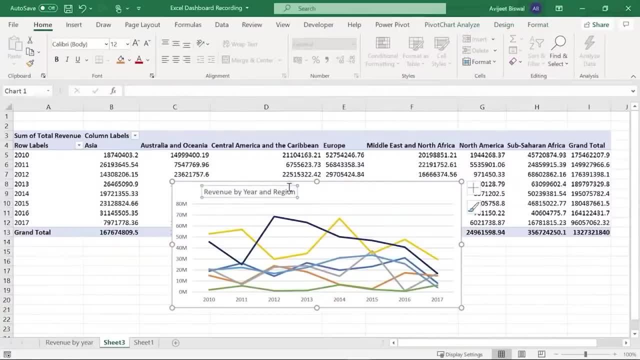 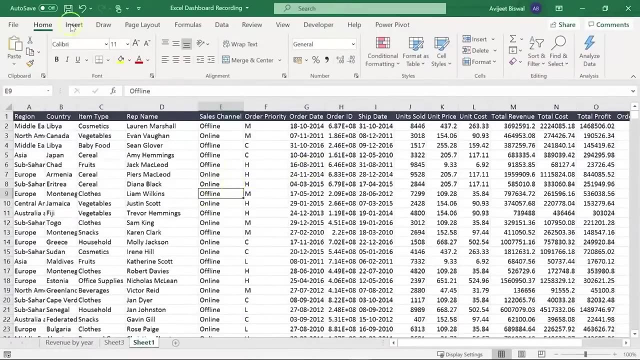 keep it to the left. all right now. we'll see the revenue and total cost by each region and we'll create a combo chart for this. so let me show you how to do it. I'll go to my datasheet. I have my cell selected, you go to insert and click on. 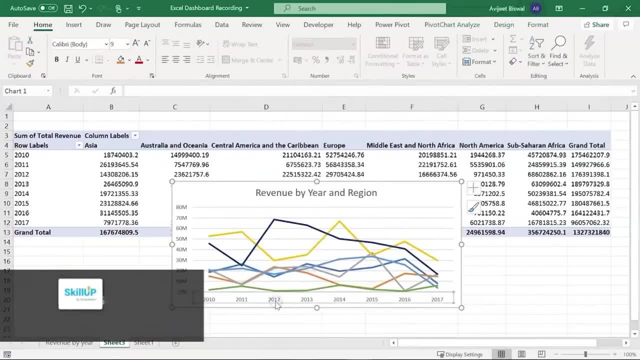 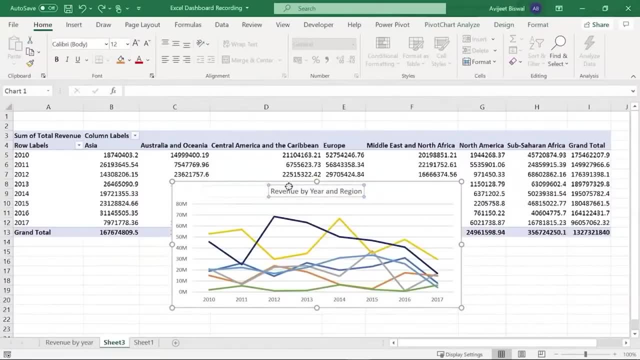 similarly, you can also edit the axis labels, also by selecting the chart title. you can also move it to left or right, or you can place it in the center as well. for the time being, let me just keep it to the left. alright, now we will see the revenue and 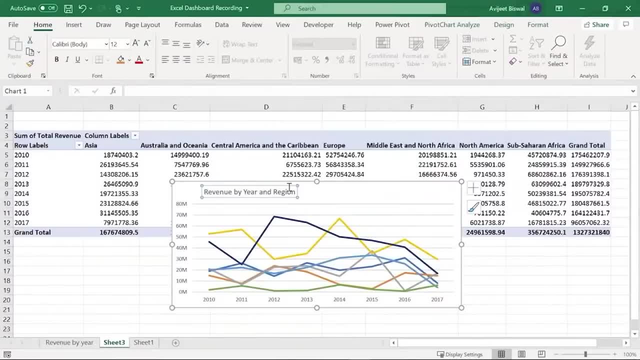 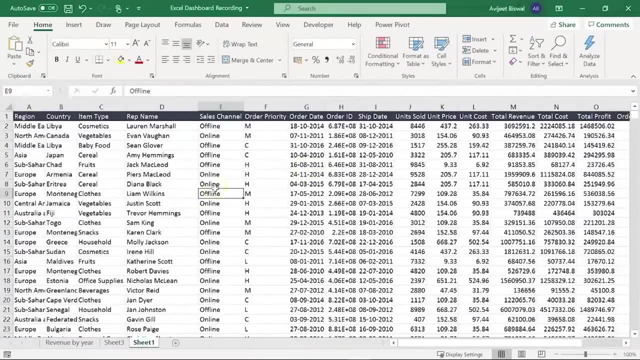 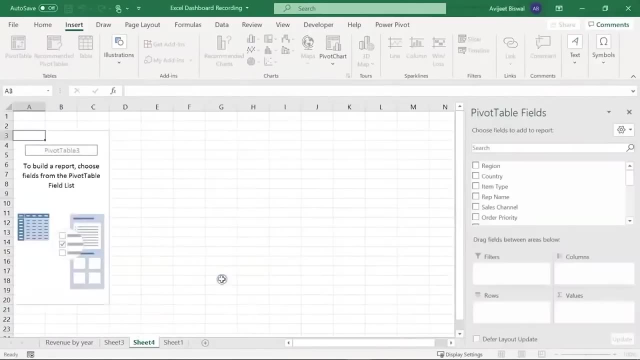 total cost by each region and we will create a combo chart for this. so let me show you how to do it. i will go to my data sheet, i have my cell selected, go to insert and click on pivot table. let me just click on ok, alright. so for this. 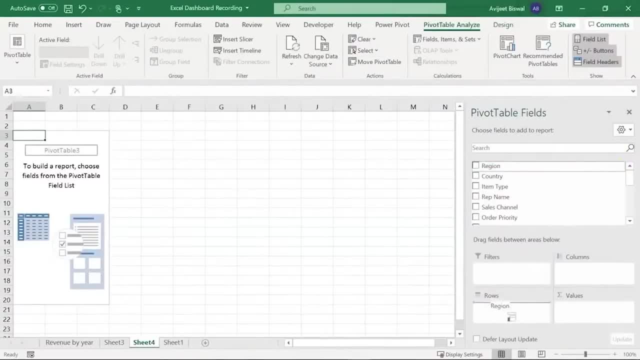 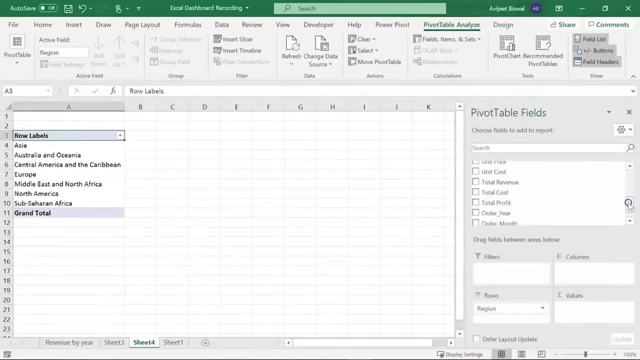 i will select my region onto rows and then i will have two columns under values. the first one is going to be total revenue and the next column will be the total cost column. alright, so here we have the pivot table ready. now, based on this pivot table, let's create our 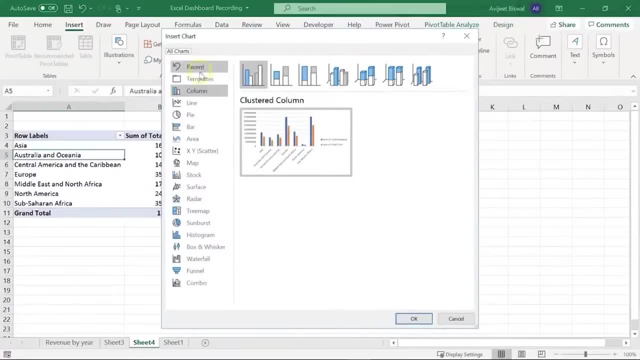 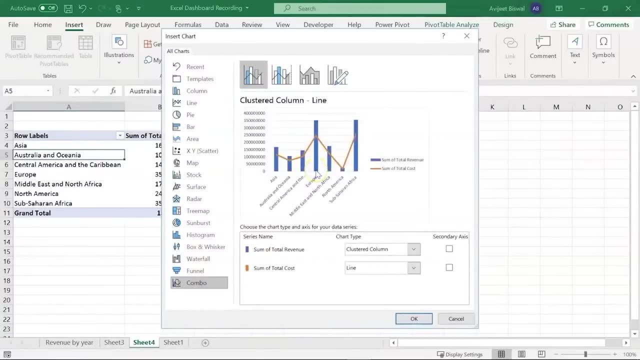 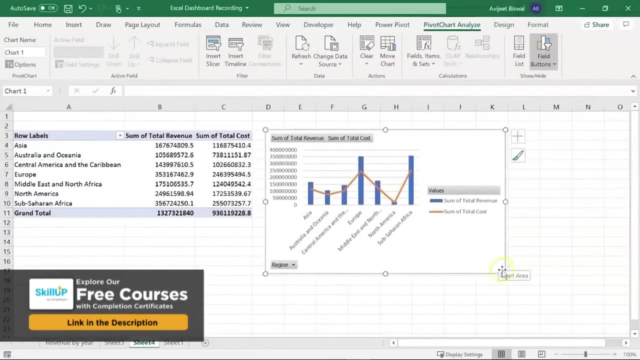 pivot chart. so i will go to recommended charts and if you see, below, at the bottom, we have combo chart. so this is the preview of the combo chart. alright, now let me just click on. ok, there you go. so we have a nice combo chart ready here now. the way to look at it is: 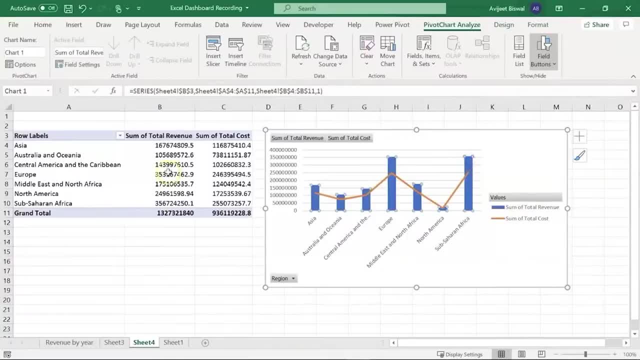 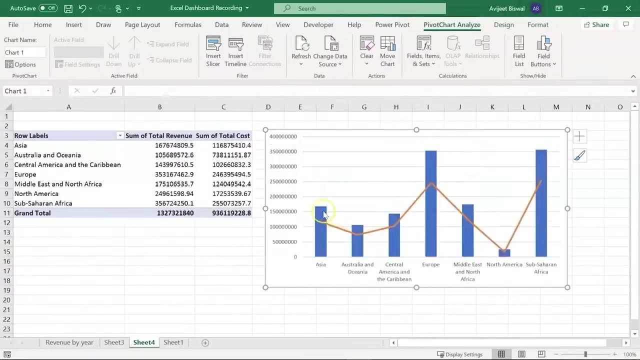 the bars represent the total revenue, which is this column. now the line represents the total cost. so let me go ahead and edit this chart a bit. so first of all, let's delete the field buttons, alright, and let's also remove the legend from here. next we will add: 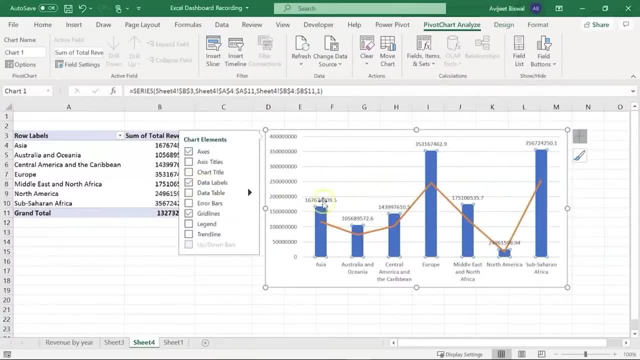 data labels. so i will click on data labels here. ok, so these are the data labels for the bars or the revenue column. now let's format the data labels in terms of millions. so i will click on this arrow. go to more options. if i scroll down, i have number. 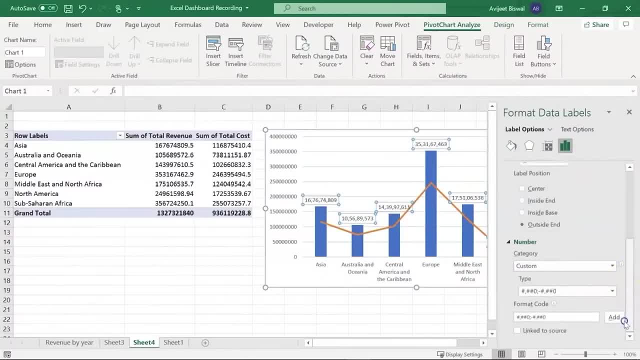 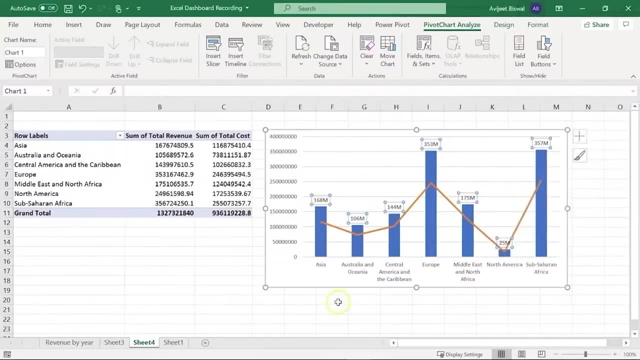 from here i will select custom and i will choose my type. that is in millions. alright, so you can see we have formatted our data. next thing: we will add a chart title. so here i will write: as revenue by region it's actually revenue and total cost by region. 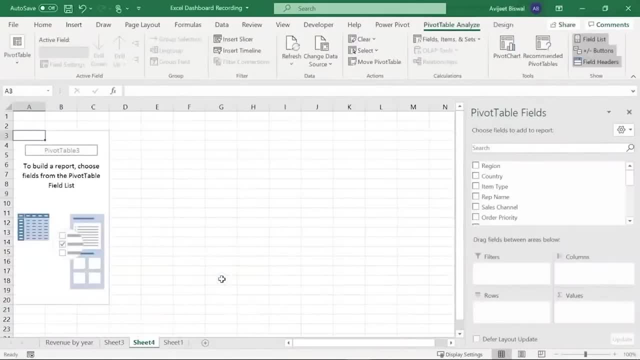 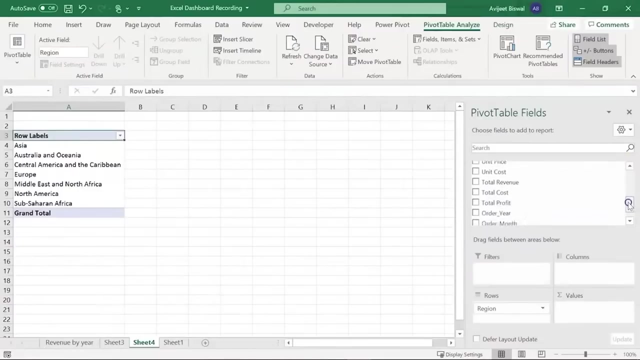 pivot table. let me just click on. ok, all right. so for this I'll select my region on to rows and then I'll have two columns under values. the first one is going to be total revenue and the next column will be the total cost column. alright, so here we have the pivot table ready now. based on this pivot table, 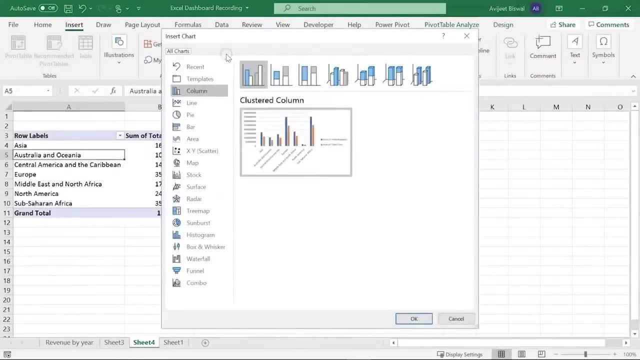 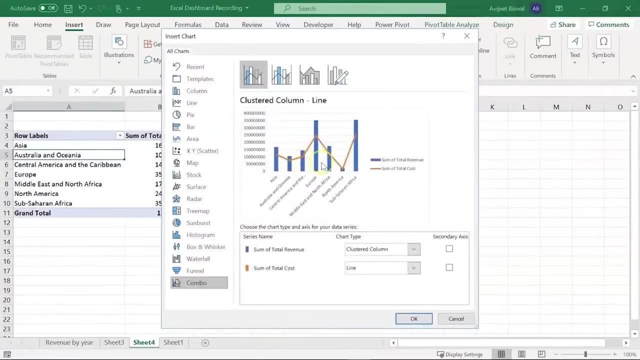 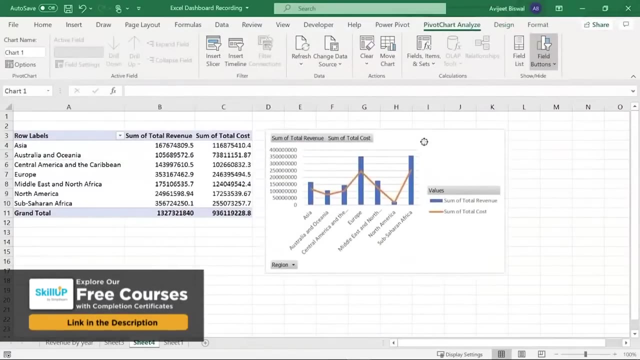 let's create our pivot chart. so I'll go to recommended charts and if you see, below at the bottom, we have combo chart. so this is the preview of the combo chart. all, right now let me just click on. ok, there you go. so we have a nice combo chart ready here now. the way to look at it is: 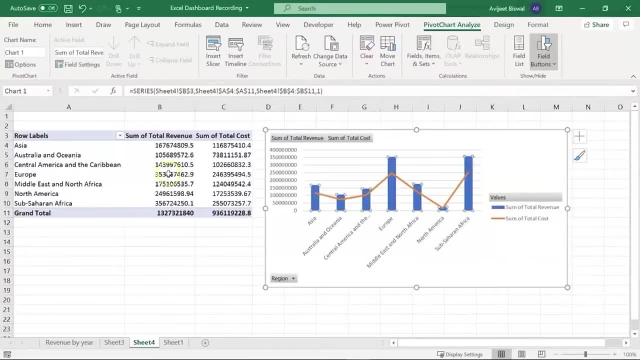 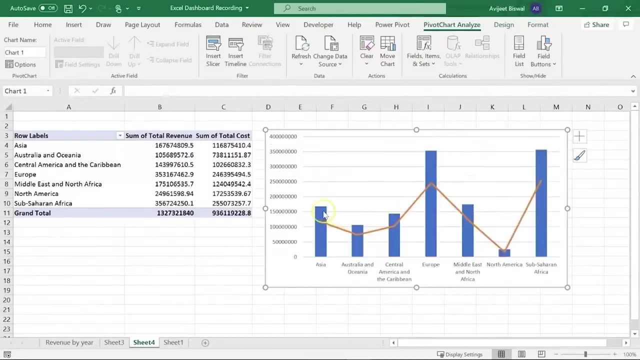 the bars represent the total revenue, which is this column. now the line represents the total cost. so let me go ahead and edit this chart a bit. so first let's delete the field buttons, all right, and let's also remove the legend from here. next we'll add data labels, so I'll click on data labels here, okay, so these 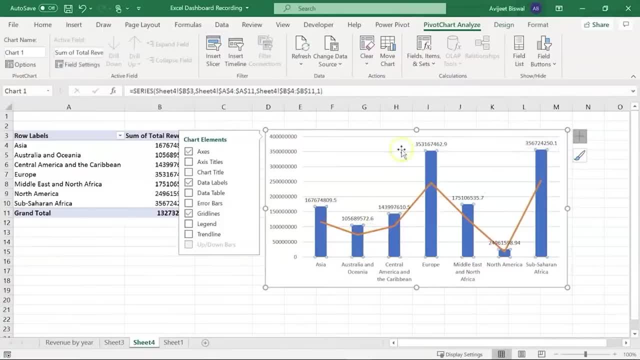 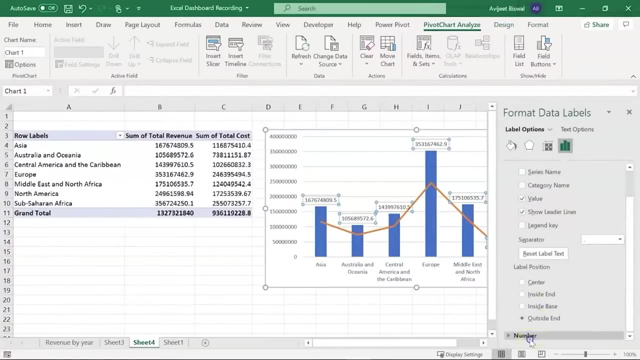 are the data labels for the bars or the revenue column. now let's format the data labels in terms of millions. so I'll click on this arrow. go to more options. if I scroll down, I have number from here. I'll select custom and I'll choose my. 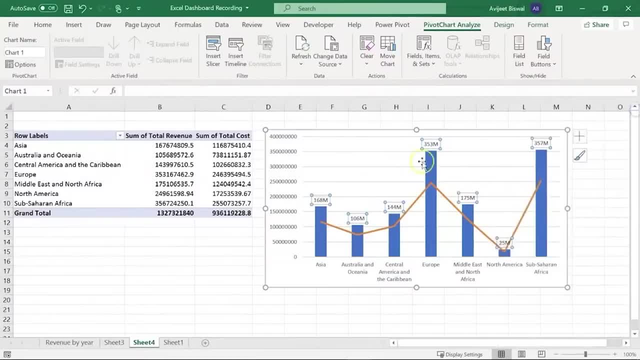 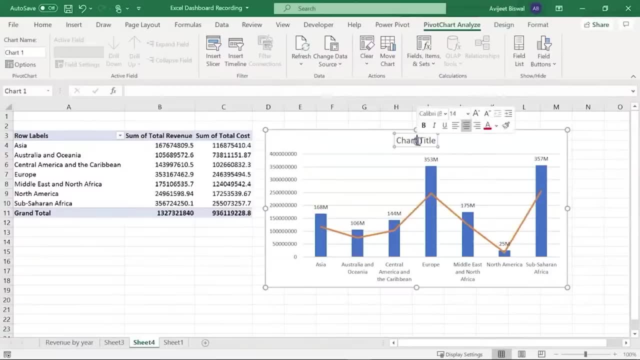 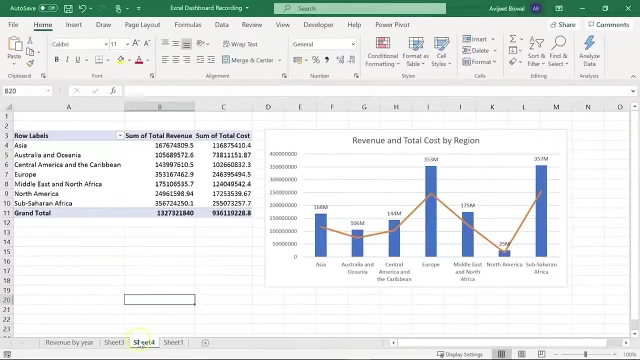 type, that is in millions. all right, so you can see we have formatted our data. next thing: we'll add a chart title. so here I'll write as revenue by region, and it's actually revenue and total cost by region. before moving ahead, let me rename the sheets as well. I'll write revenue and total cost. similarly, sheet 3 also. I'm 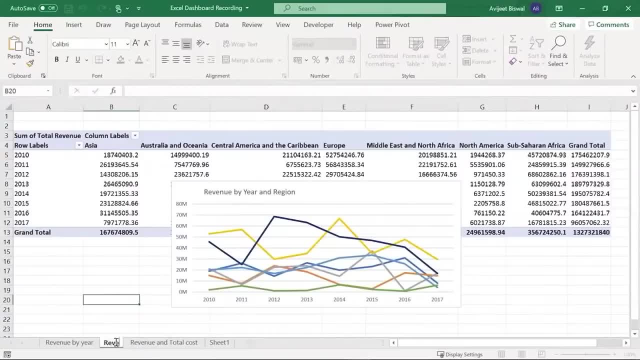 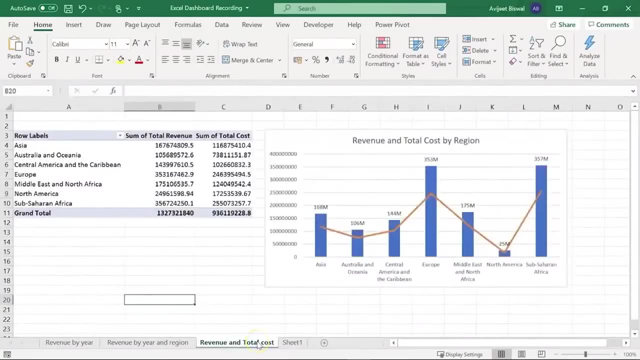 going to rename it as revenue by region, here and region, so this makes your sheet more readable. all right, now moving ahead. next we are interested to get the revenue generated by order priority, and for this we are going to create a pie chart. so let's go to the data sheet and 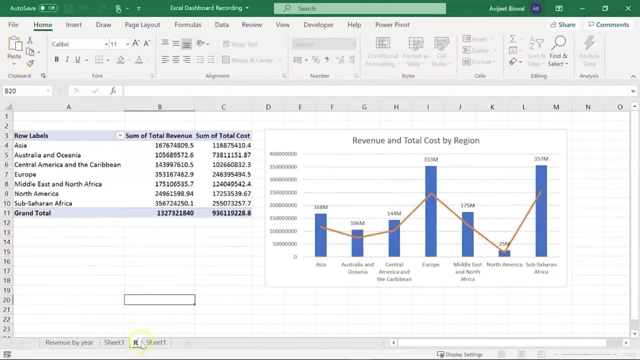 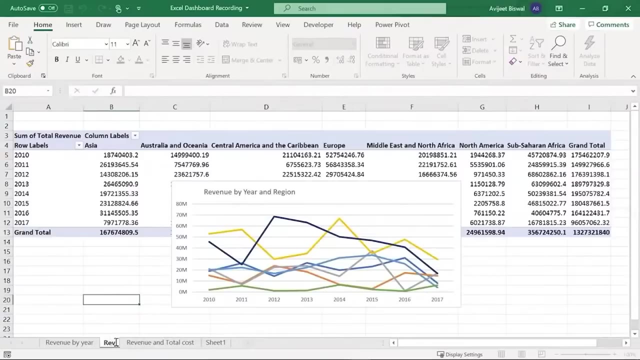 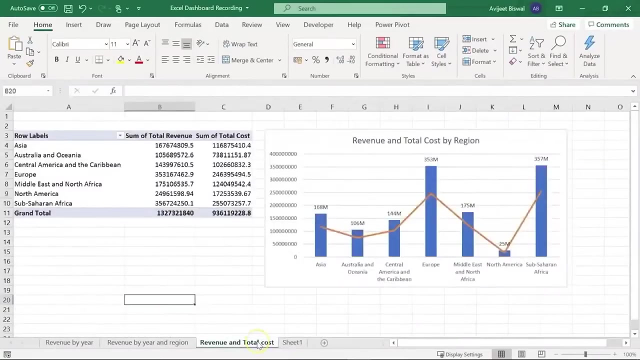 before moving ahead, let me rename the sheets as well. i will write revenue and total cost. similarly, sheet 3. also, i am going to rename it as revenue by year and region, so this makes your sheet more readable. alright, now moving ahead. next, we are interested to get the revenue generated. 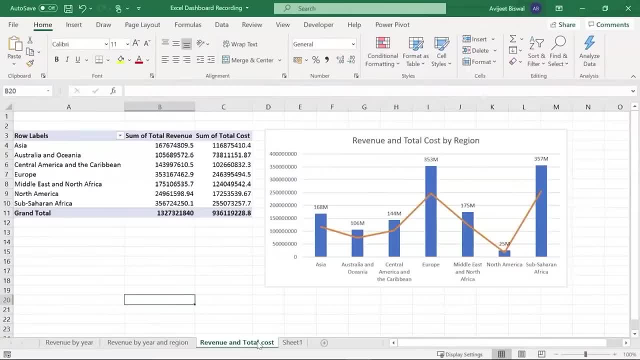 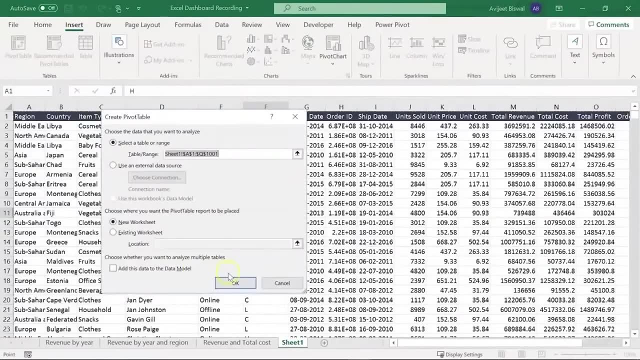 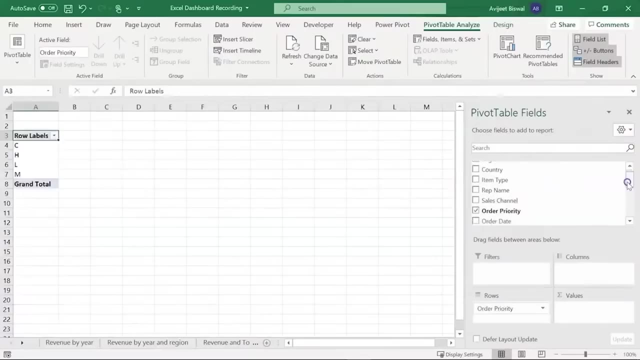 by order priority, and for this we are going to create a pie chart. so let's go to the data sheet and create our pivot table. first i click on ok. now i will select order priority. under rows, and under values i will select total revenue. so this is a very simple. 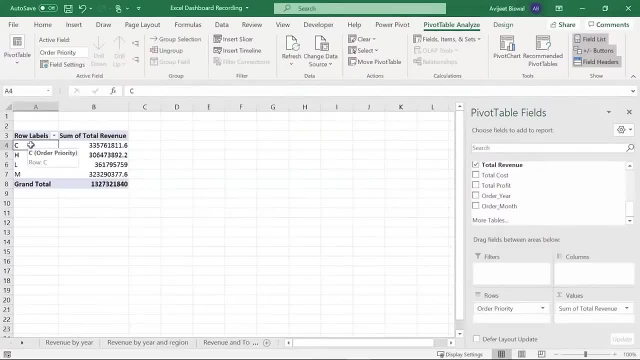 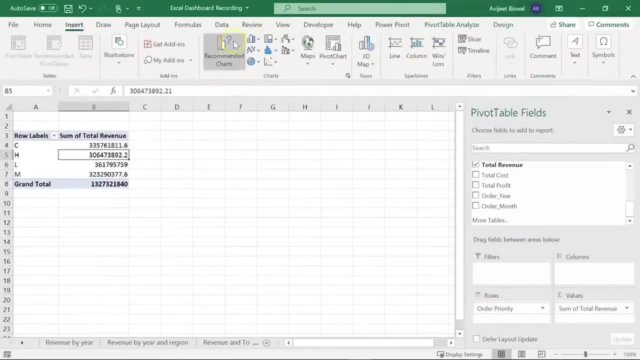 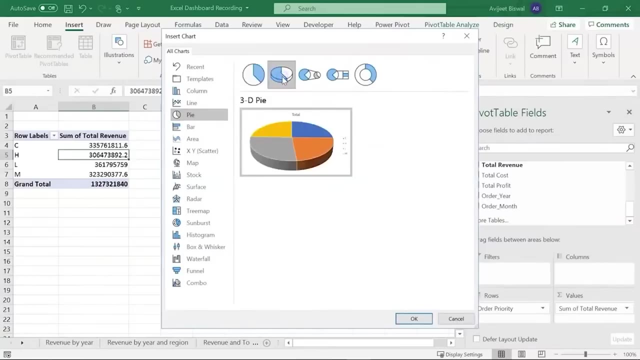 pivot table. so you have your order priority. so c is for critical, h is for high, l is for low and m is for medium. now, based on this, let's create a pie chart. so i will go to recommended charts and here you have pie chart. i want to select. 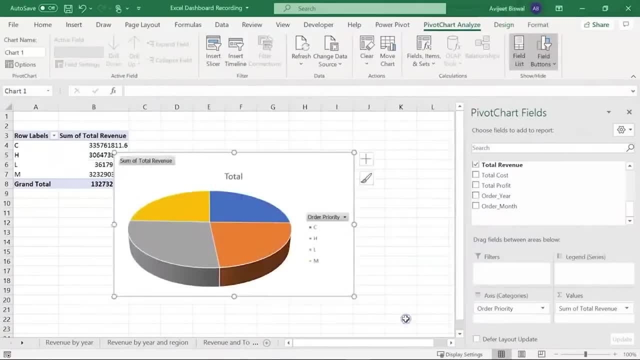 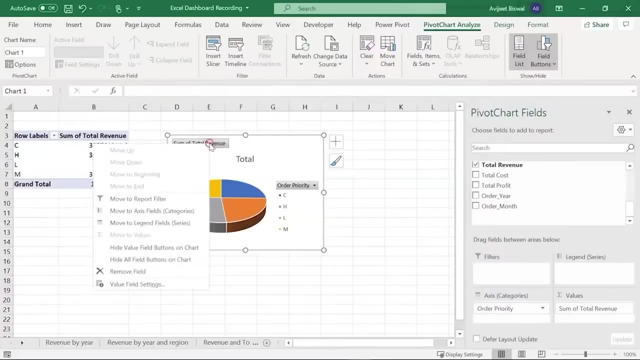 this 3d type of pie chart and i will click on ok. alright, so we have our pie chart ready. let me just resize it and from here i will remove the field buttons, and i also don't need the legend, so i will delete this as well, alright. 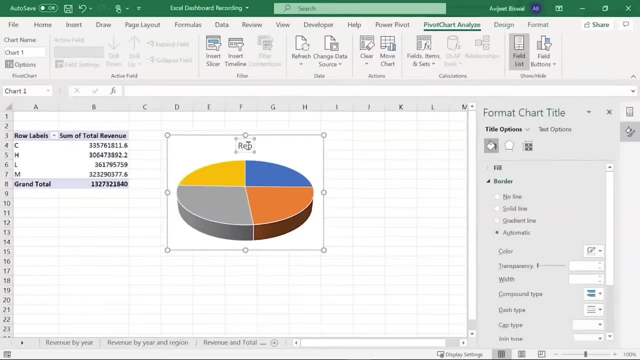 now let's give a chart title, so this is going to be revenue by order priority. now let's add our data labels. i will check this option. ok, now let's again format this in terms of millions. so here i will click on the last option. i will go to numbers under. 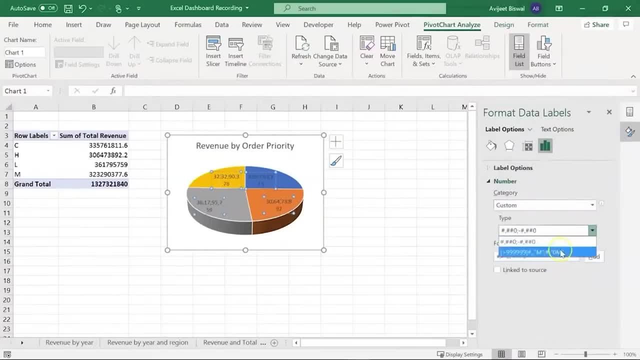 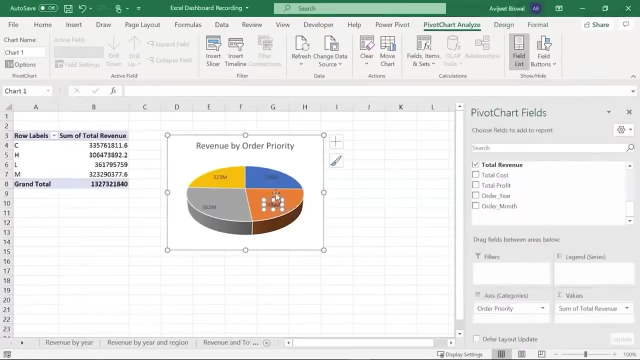 category. i will select custom, and my type is going to be in terms of millions. there you go. let me close this. i will just move this to the center. alright, now, if you want, you can change the color of the text as well. so let's have it in white color. 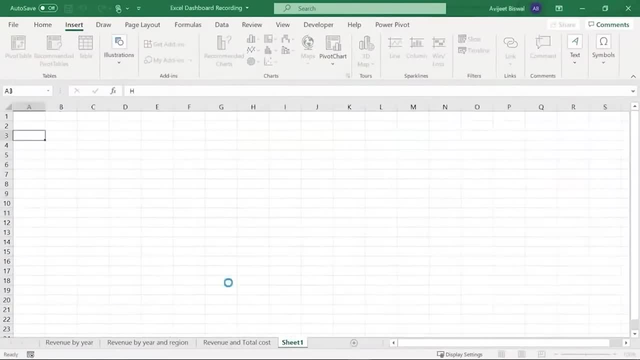 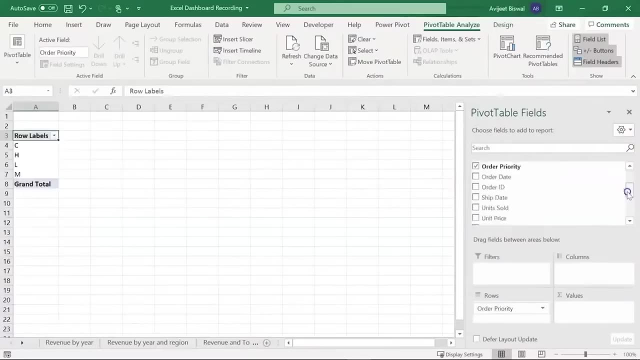 create our pivot table. first click on OK and then we will need to create the chart. Now I'll select order priority under rows and under values I'll select total revenue. So this is a very simple pivot table. So you have your order priority. 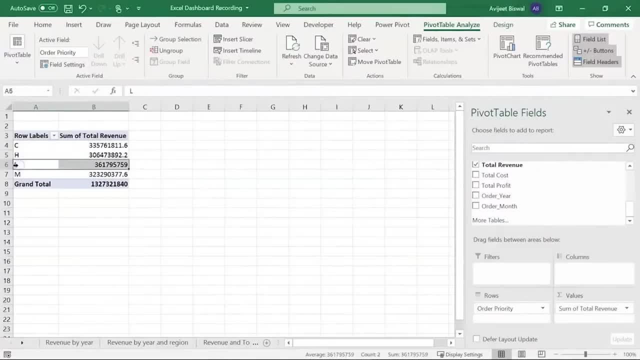 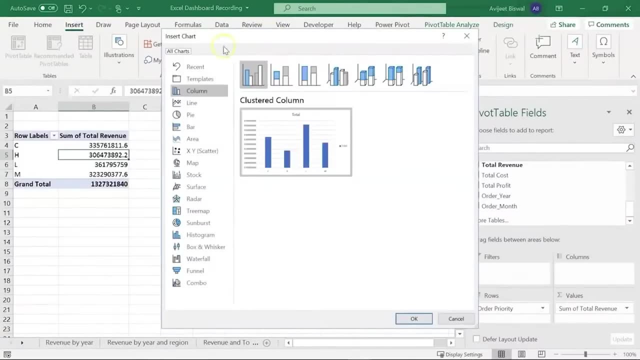 So C is for critical, H is for high, L is for low and M is for medium. Now, based on this, let's create a pie chart. So I'll go to recommended charts and here you have pie chart. I want to select this 3D type of pie chart and I'll click on OK. 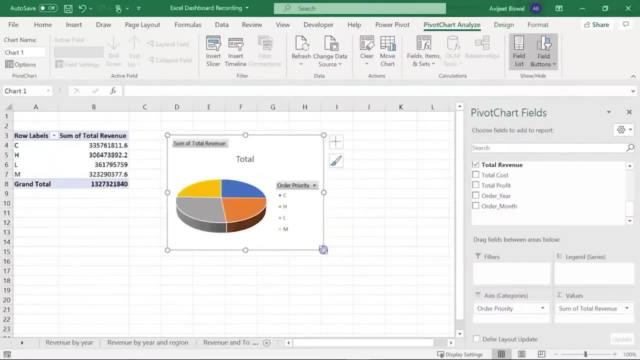 Alright, so we have our pie chart ready. Let me just resize it, and from here I'll remove the field buttons, and I also don't need the legend, So I'll delete this as well. Alright, now let's give a chart title. 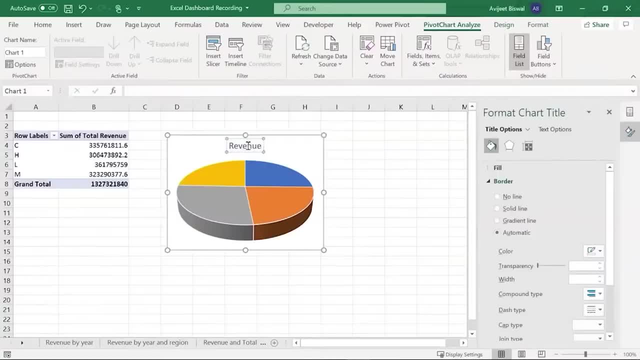 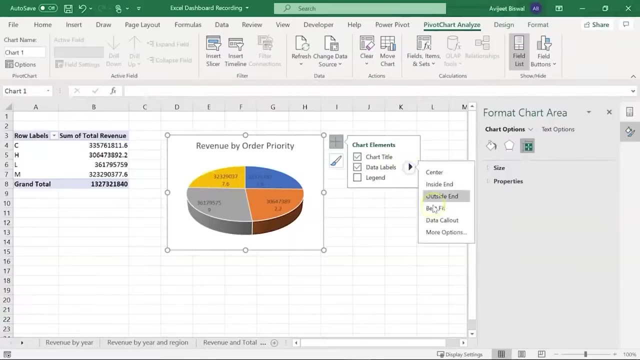 So this is going to be revenue by order priority. Now let's add our data labels. I'll check this option. Okay, now let's again format this in terms of millions. So here I'll click on the last option. 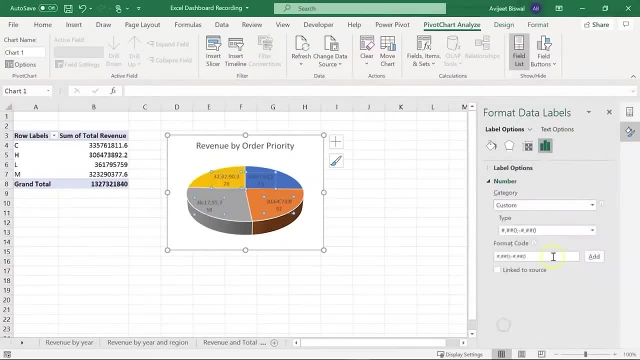 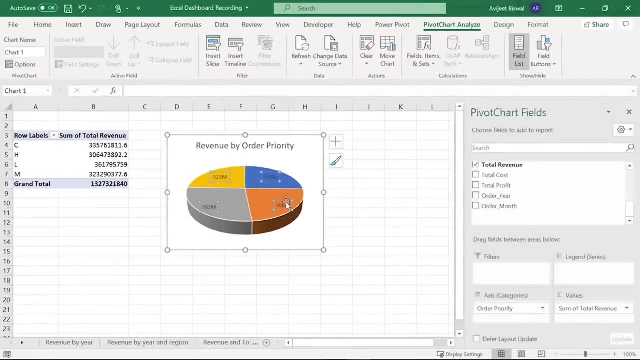 I'll go to numbers under category. I'll select custom and my type is going to be in terms of millions. There you go, Let me close this, I'll just move. I'll move this to the center. Alright, Now, if you want, you can change the color of the text as well. 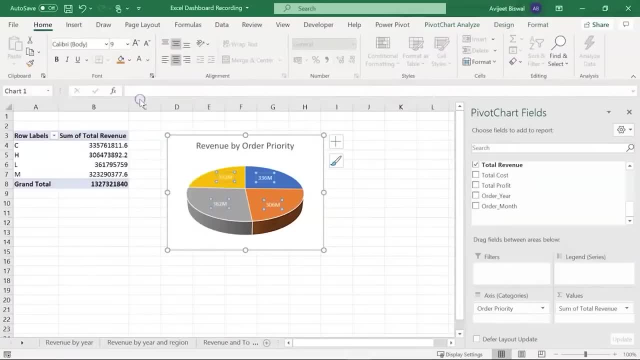 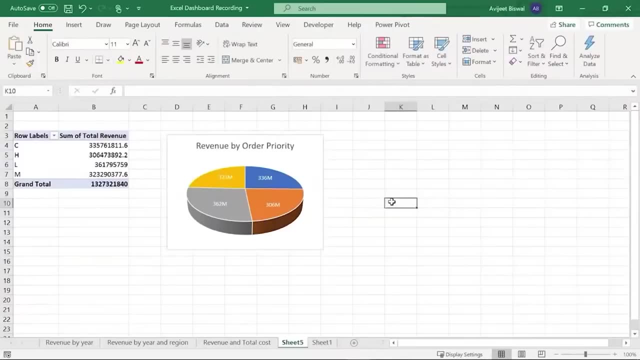 So let's have it in white color and see how it looks. Okay, so this looks pretty decent, Cool. Now moving to our next report. So this time We are going to find the total revenue by countries, So we have multiple countries present in our data set. 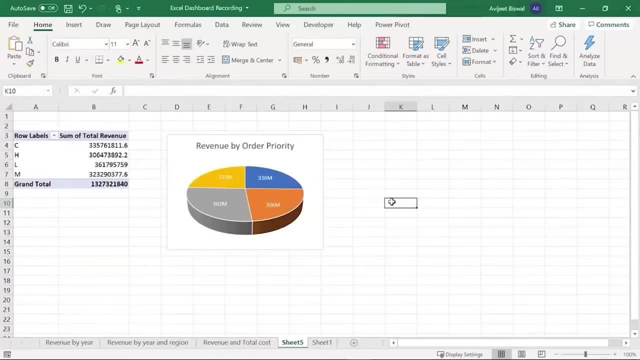 We want to visualize the revenue generated in each country. So for this we are going to create a horizontal bar chart. So let me show you how to do it. But before moving ahead, let me just rename this sheet. So I'll write revenue by. I'll just put OP, which stands for order priority. 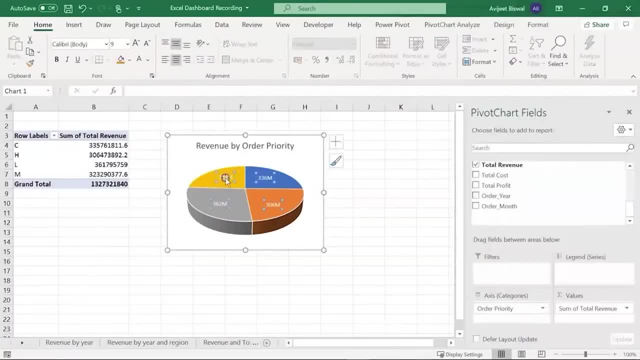 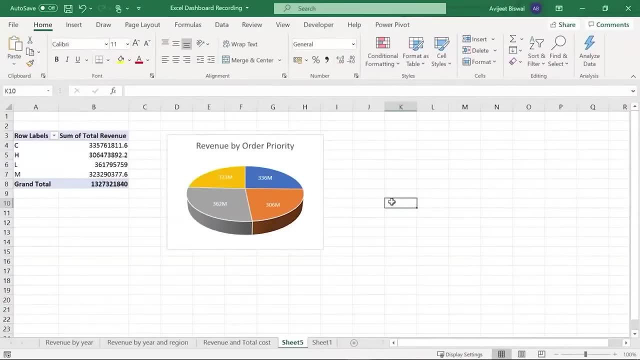 and see how it looks. ok, so this looks pretty decent, cool. now moving to our next report. so this time we are going to find the total revenue by countries, so we have multiple countries present in our data set. we want to visualize the revenue generated in each country. 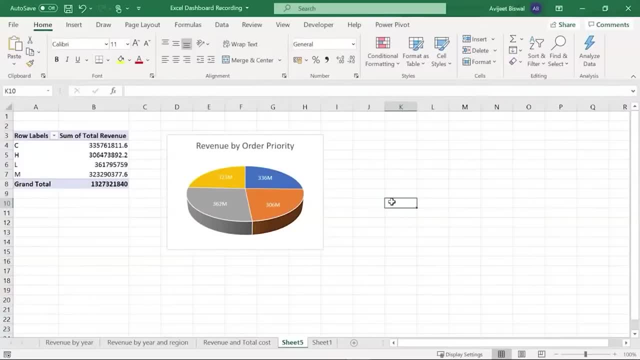 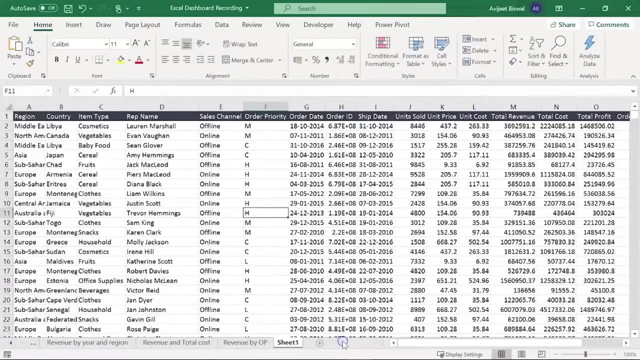 so for this we are going to create a horizontal bar chart. so let me show you how to do it. but before moving ahead, let me just rename this sheet, so i will write revenue by. i will just put op, which stands for order priority. alright, now let's create. 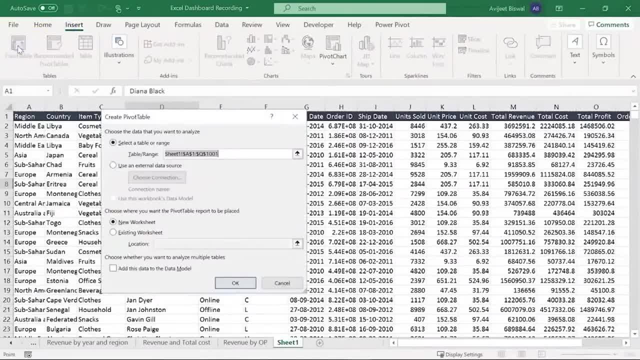 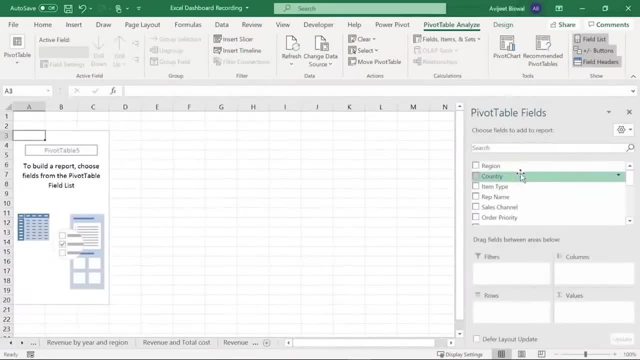 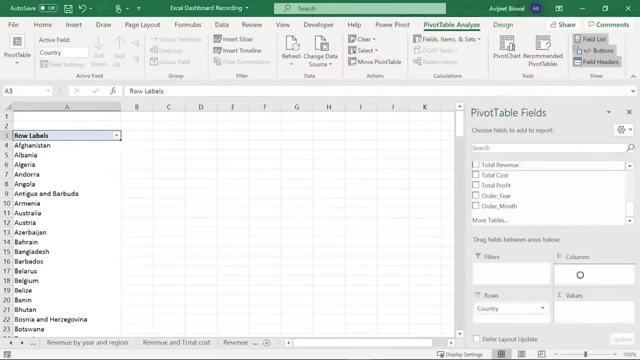 our horizontal bar chart. i will go to insert, click on pivot table and select: ok, so i want my revenue based on different countries, so i will select country and put it under rows, and then i will choose total revenue and place it under values. so here you have the different country names. 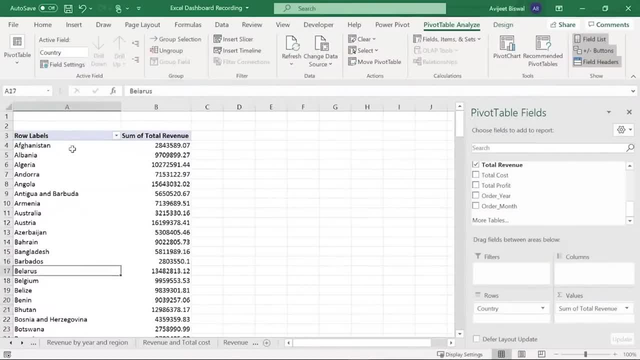 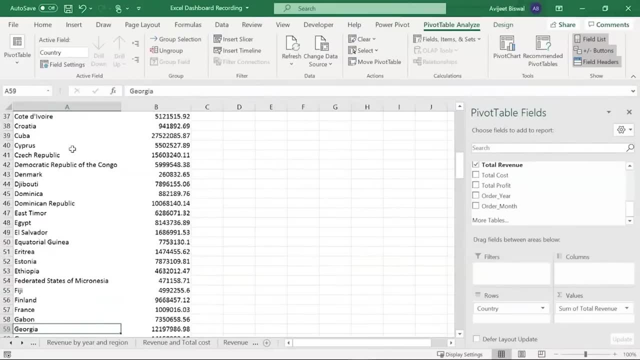 you have afghanistan, there is albania. let me scroll down. you have bangladesh. there are a number of countries. you have czech republic, there is estonia, france, gabon. similarly, if you scroll down, we have india, there is jamaica, italy. 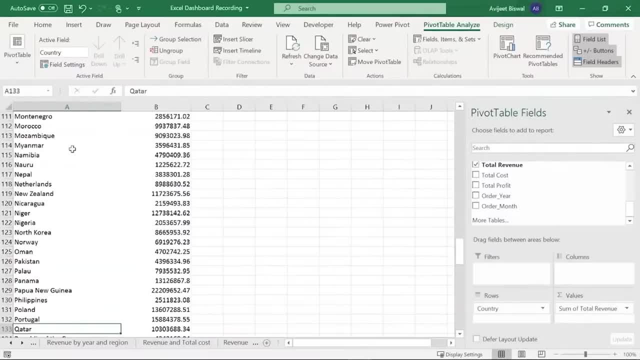 and all the way to the bottom if you go. we have new zealand, there is netherlands, philippines, portugal. we also have singapore, lots and lots of countries. we have the uae, united states of america, zimbabwe and others. alright, let me go up. so, based on this pivot, 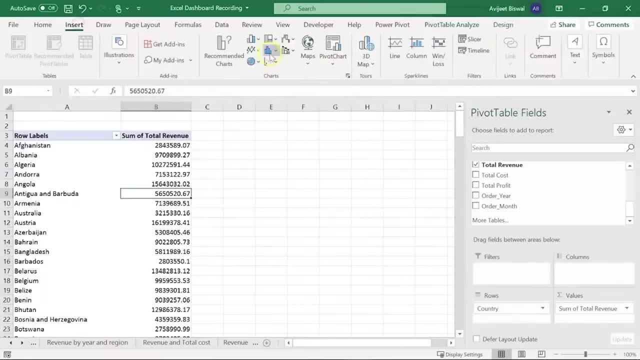 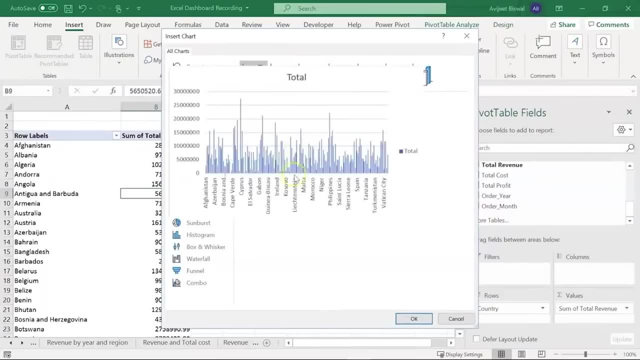 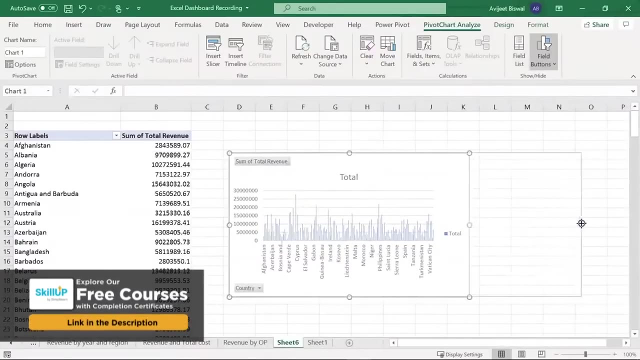 table. let's create our pivot chart. so i will go to insert and select recommended charts from here. i am going to select the column chart. you can see the preview here and let me click on ok, alright. so here you can see the different country names at the bottom and 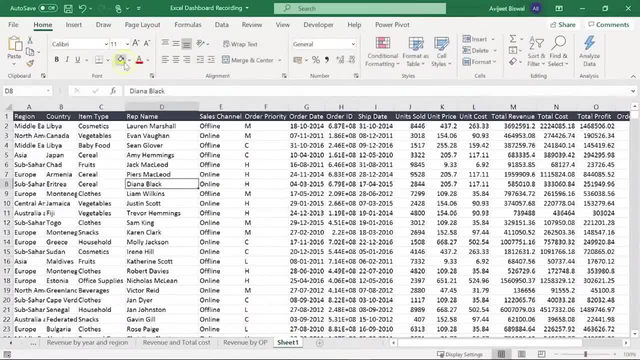 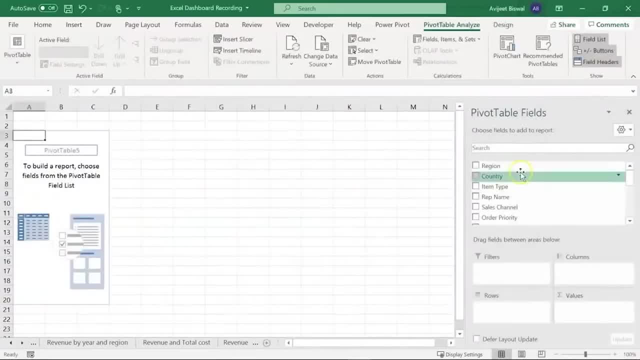 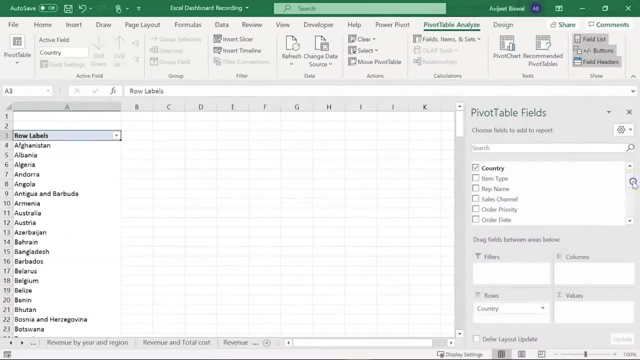 Alright, Now Let's create our horizontal bar chart. I'll go to insert, click on pivot table and select: okay, So I want my revenue based on different countries. So I'll select country and put it under rows and then I'll choose total revenue and place it under values. 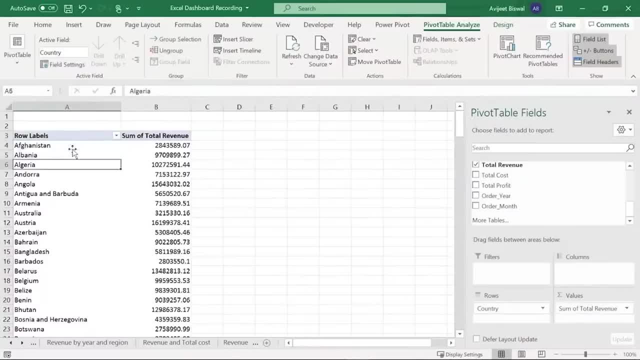 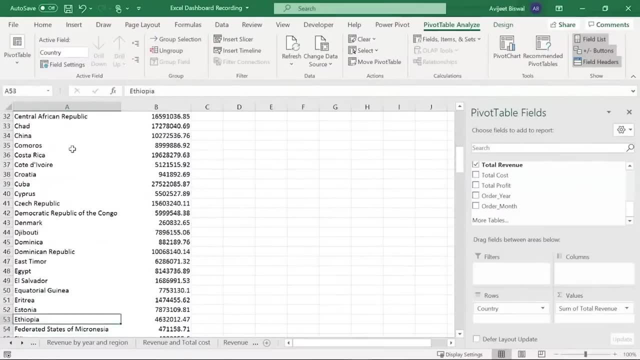 So here you have the different country names. We have Afghanistan, There's Albania- Let me scroll down. You have Bangladesh. There are A number of countries. you have Czech Republic, there's Estonia, France, Gabon. Similarly, if you scroll down, we have India, there's Jamaica, Italy and all the way to the bottom. 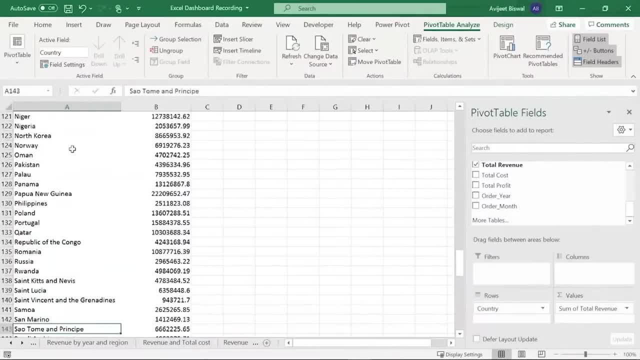 If you go, we have New Zealand, there's Netherlands, Philippines, Portugal, We also have Singapore, lots and lots of countries. We have the UAE, United States of America, Zimbabwe and others. Alright, Let me go up. So, based on this pivot table, let's create our pivot chart. 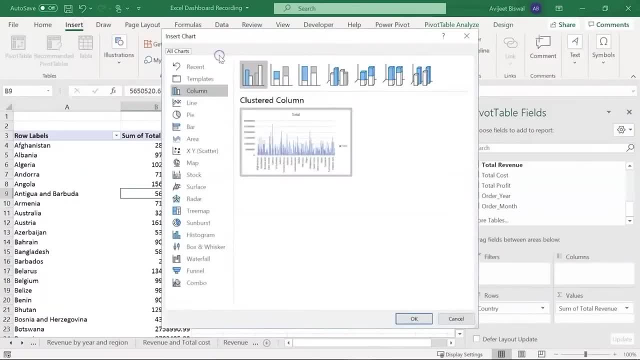 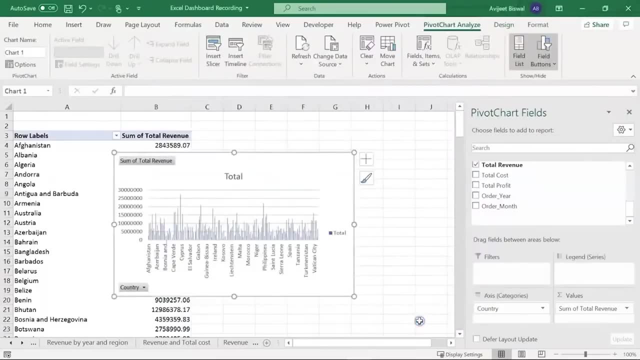 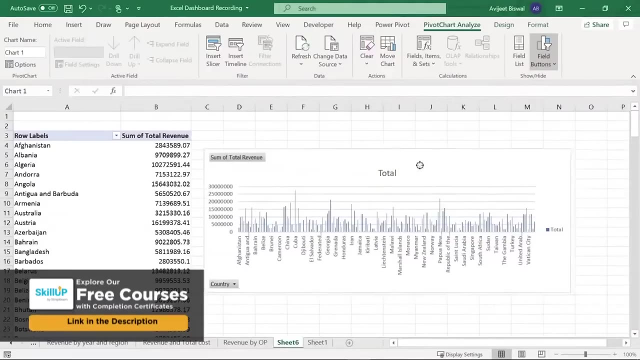 So I'll go to insert and select recommended charts From here. I'm going to select the column chart. You can see the preview here and let me click on. okay, Alright. So here you can see the different country names at the bottom and the revenue for each. 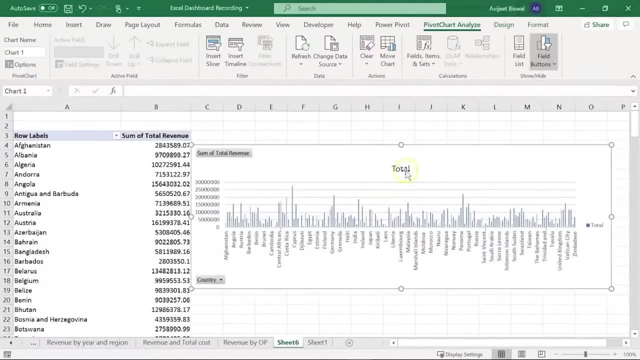 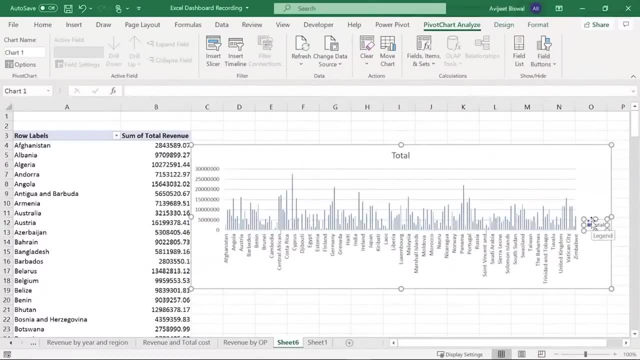 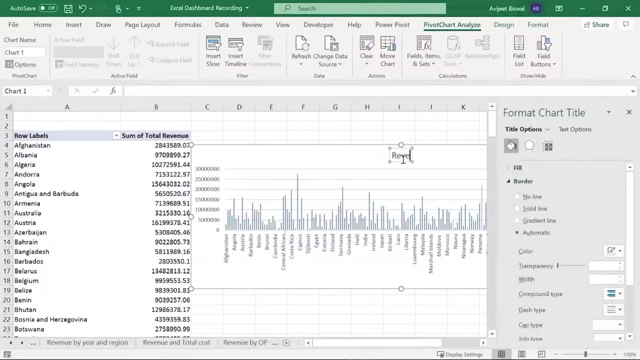 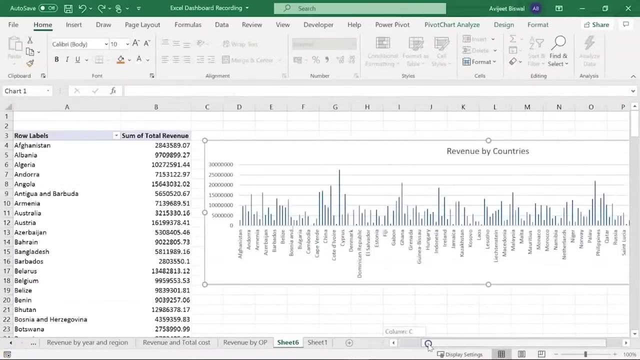 of the countries. Let's go ahead and edit this chart, Alright. so first of all, I'll delete the field buttons, okay, and let me also remove the legend. here I'll write: revenue by countries is going to be my chart title. okay, let's format this chart. 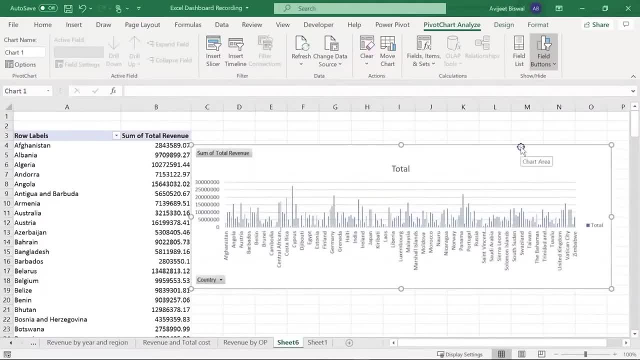 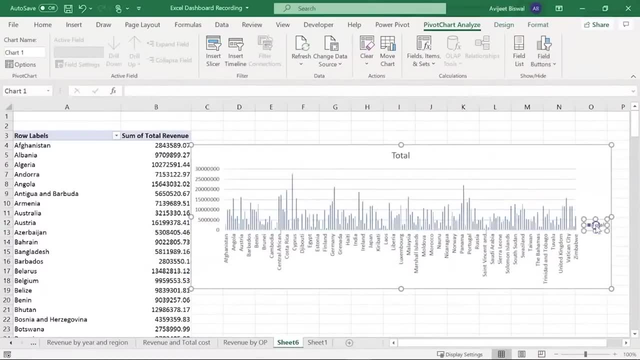 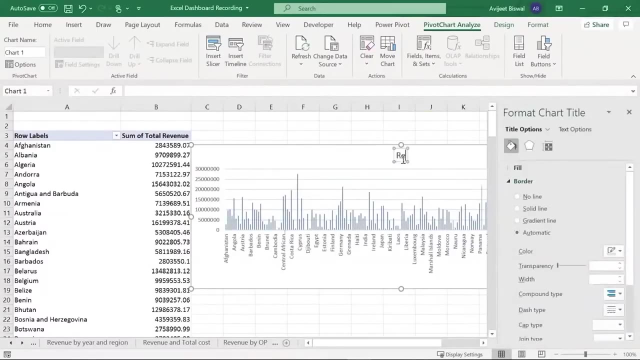 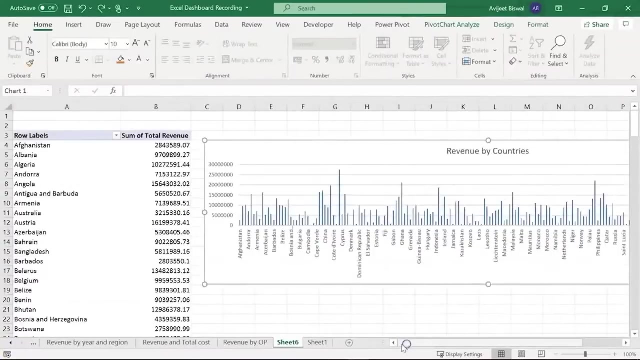 the revenue for each of the countries. let's go ahead and edit this chart. so first of all, i will delete the field buttons, ok, and let me also remove the legend. here i will write revenue by countries. this is going to be my chart title. ok, let's format this chart a little more. 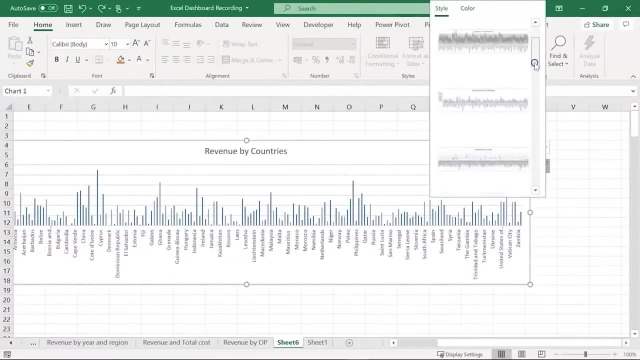 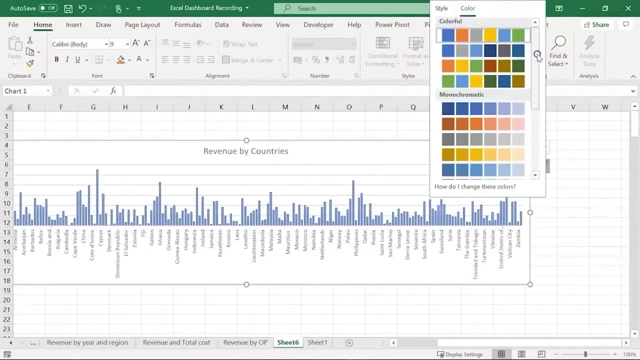 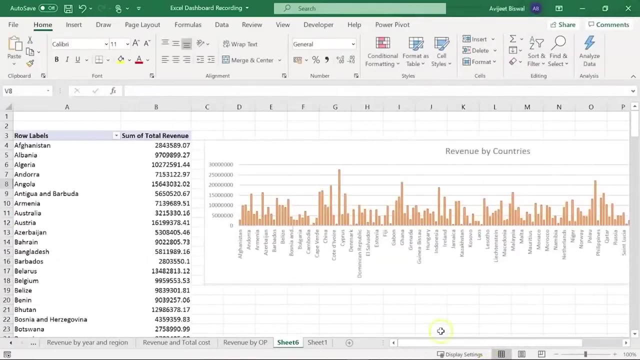 so i will click on this option and we will select a new style. let's say, i will select style 6. ok, and let me now go under colors and we will select the color of the bars. so let's choose this color. ok, so you have a horizontal. 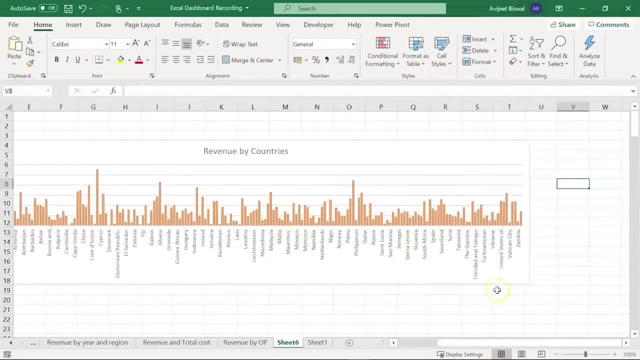 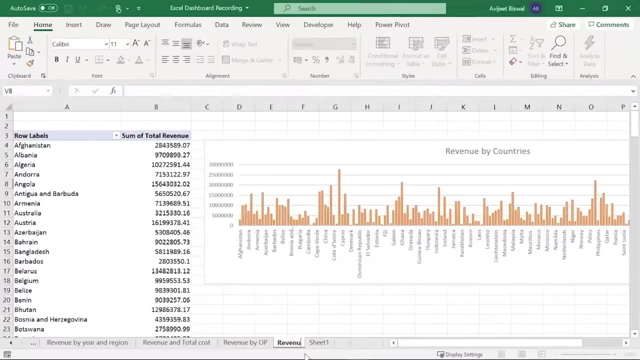 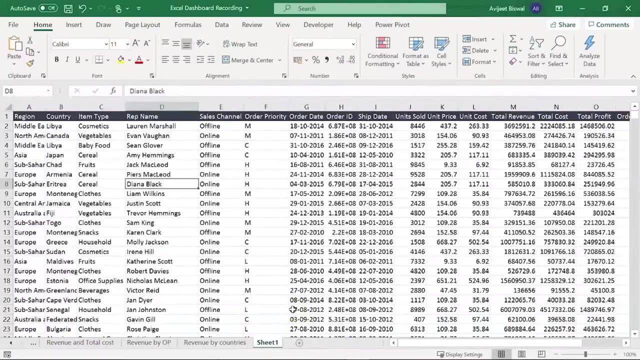 column chart ready and at the bottom you can see the different country names and we have the revenue. ok, cool, now let me go ahead and rename this sheet, so i will write revenue by countries and hit enter ok, and finally, we will create another report, which is going to be: 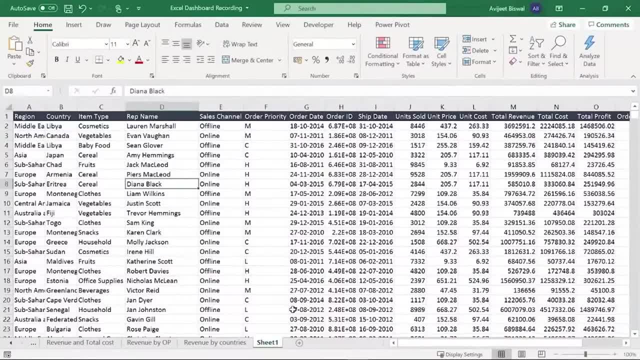 part of our revenue dashboard and this is revenue by items, so we will visualize our revenue for different items present in the table. so, if you see this, we have cosmetics, vegetables, cereal, fruits. there's cloths, snacks, households and other products as well. so let's check the revenue. 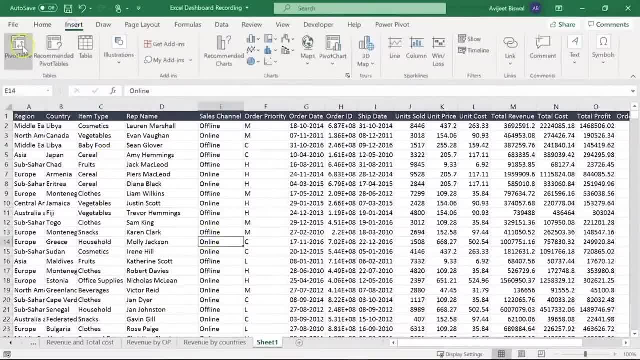 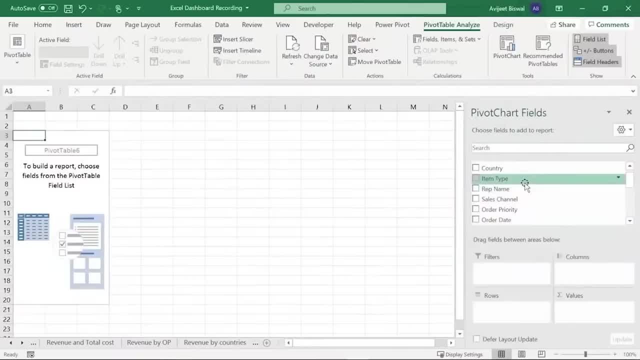 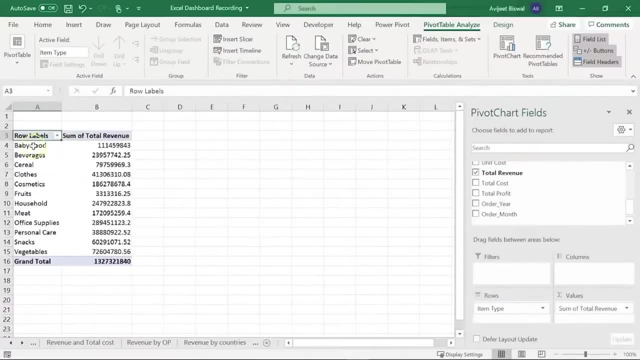 for each of these items. so we will continue the same drill. i will create my pivot table on a new worksheet and this time i am going to drag item type under rows and we will have the total revenue under values. so here on the left of the table, you can see we have. 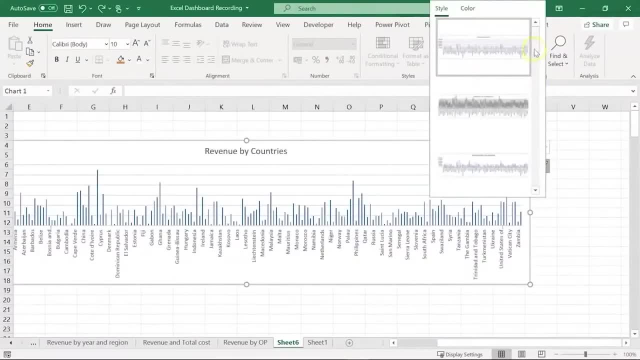 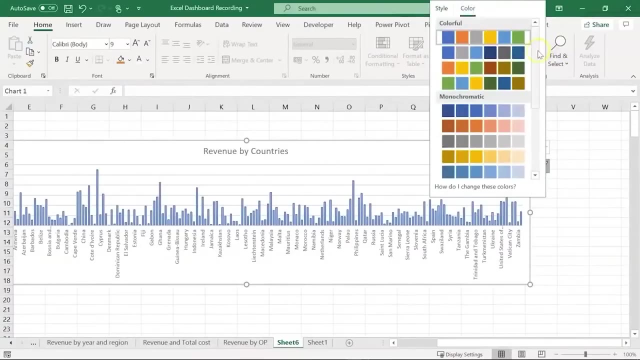 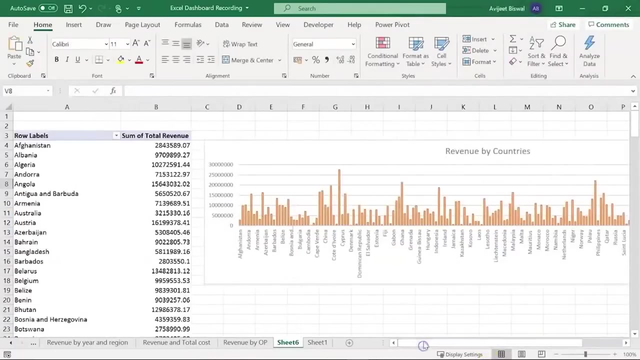 a little more. so I'll click on this option and we'll select a new style. let's say I'll select style 6. okay, and let me now go under colors and we'll select the color of the bars. so let's choose this color, okay? so you have a horizontal column chart ready and at the bottom you can see the. 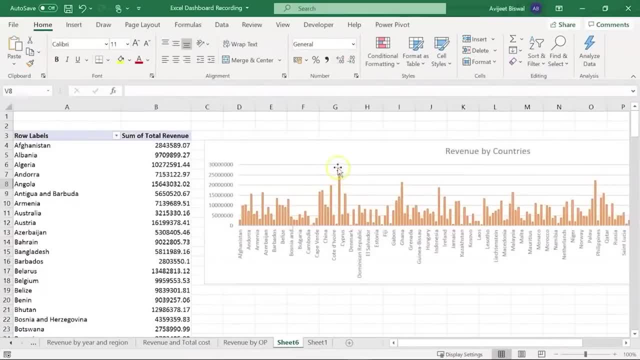 different country names and we have the revenue. cool, now let me go ahead and rename the sheet, so I'll write revenue by countries and hit enter okay, and finally we'll create another report which is a product name. okay, now let's complete the report. we also have another component named. 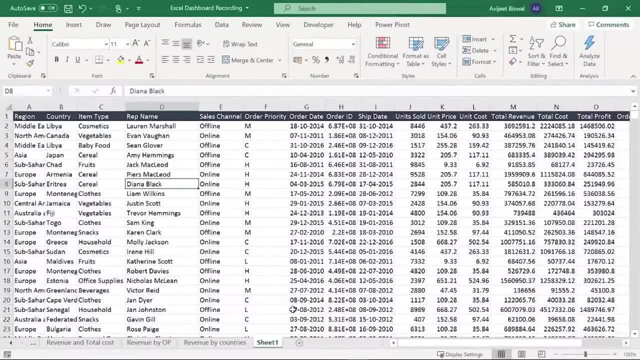 content method, whichた I can then just provide the opening menu with potential information going to be part of our revenue dashboard, and this is revenue by items, so we'll visualize our revenue for different items present in the table. so, if you see this, we have cosmetics, vegetables, cereal, fruits, there's cloths. 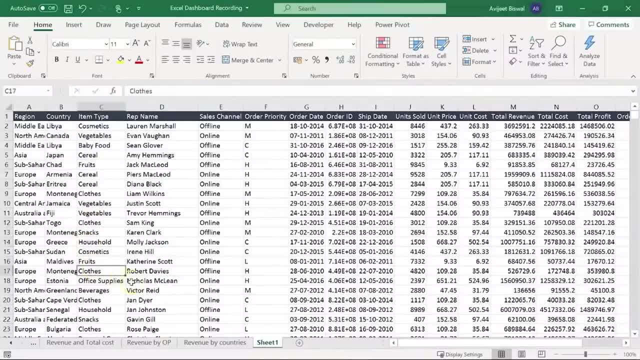 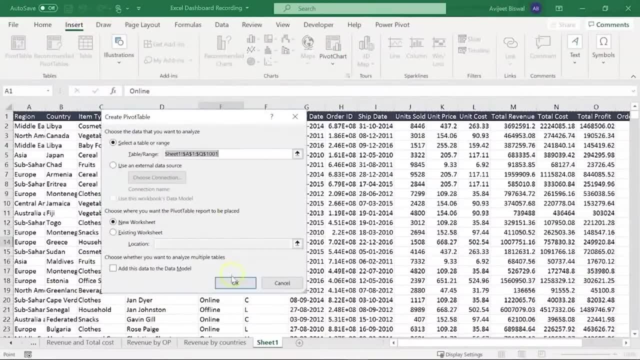 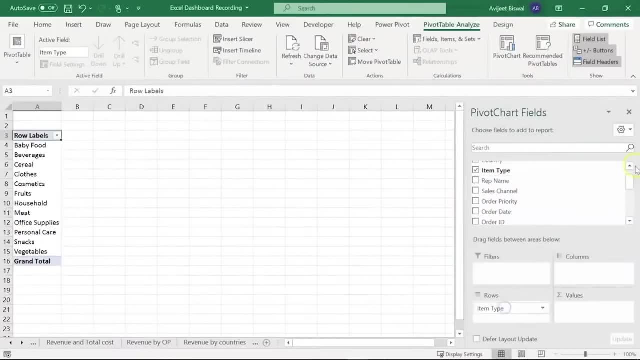 snacks, households and other products as well. so let's check the revenue for each of these items. so we'll continue the same drill. I'll create my pivot table on a new worksheet and this time I'm going to drag item type under rows and we'll have the total revenue under values. so here on the left of the table, you can. 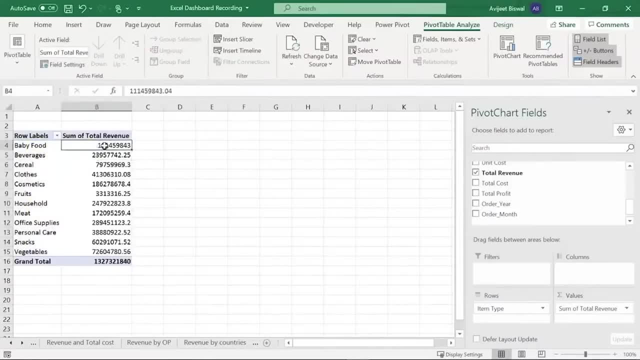 see we have the different item names and then we have the total revenue. so let me just short this total revenue from largest to smallest so you can see here: office support supplies meet the highest amount of revenue, followed by household, then cosmetics and fruits meet the lowest amount of revenue. I'll click on this go. 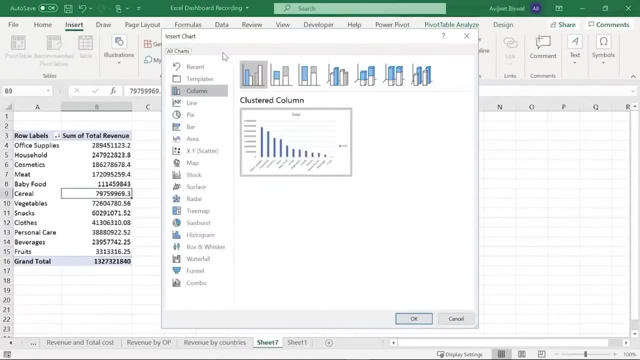 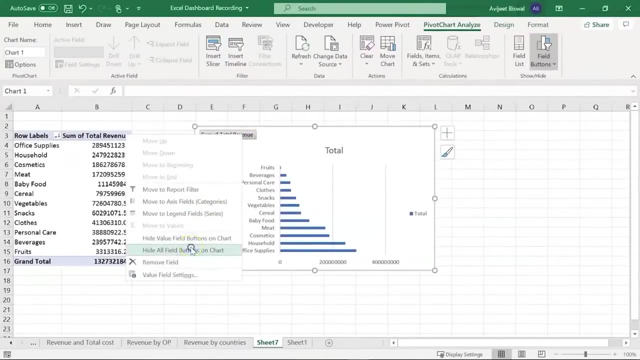 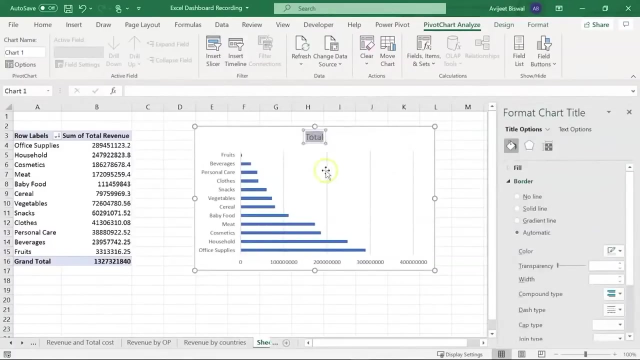 to insert and select recommended charts. this time I'm going to create a bar chart, so this is how my bar chart is going to look like. I'll select: ok, alright, now let's format this chart a bit. I'll delete the field by buttons and I'll delete the legend as well, and let's edit the chart title. so 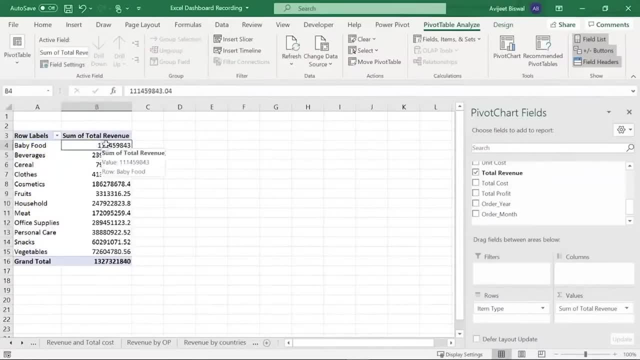 the different item names and then we have the total revenue. so let me just sort this total revenue from largest to smallest so you can see here office supplies meet the highest amount of revenue, followed by household, then cosmetics and fruits meet the lowest amount of revenue. i will click on this. 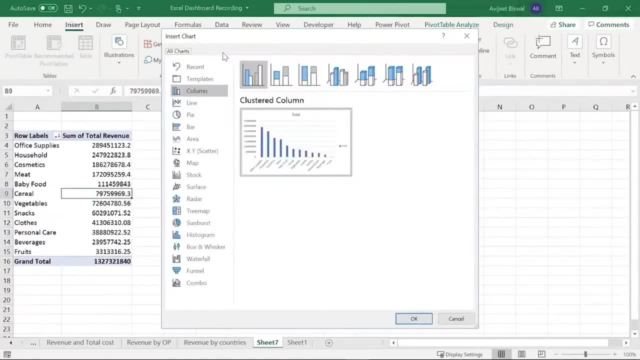 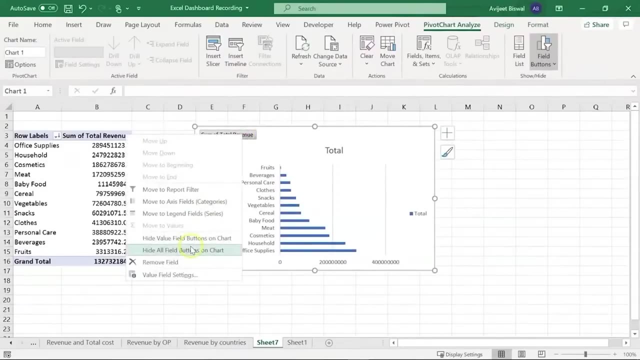 go to insert and select recommended charts. this time i am going to create a bar chart, so this is how my bar chart is going to look like. i will select: ok, alright, now let's format this chart a bit. i will delete the field buttons and i will delete. 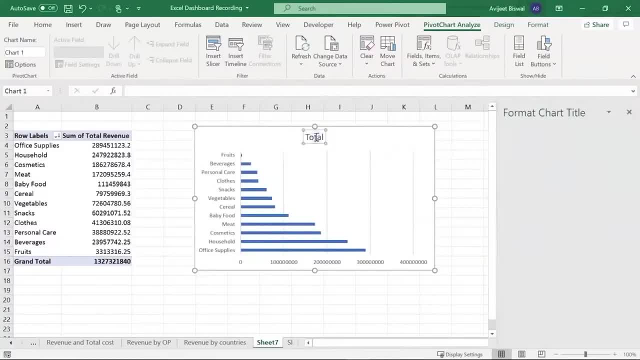 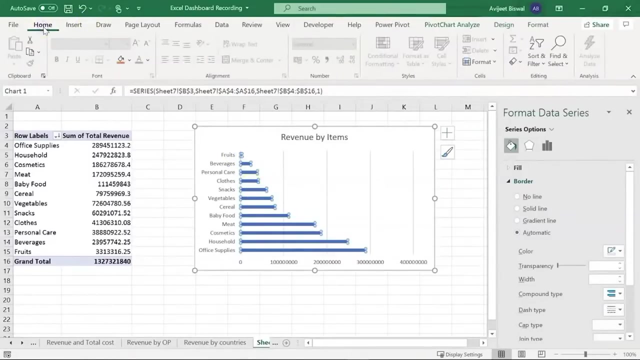 the legend as well, and let's edit the chart title. so this is going to be revenue by items- cool. we also want to change the color of the bars, so i have selected all the bars. i will go to my home tab and here let's say i: 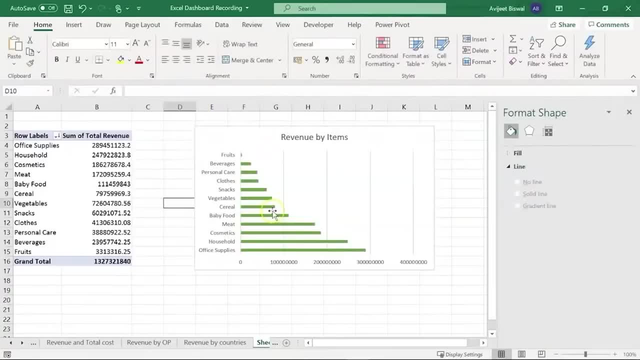 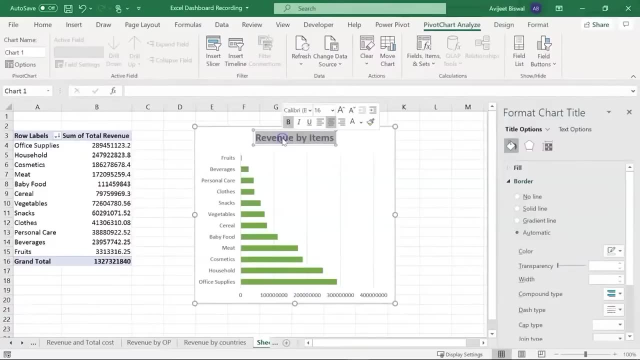 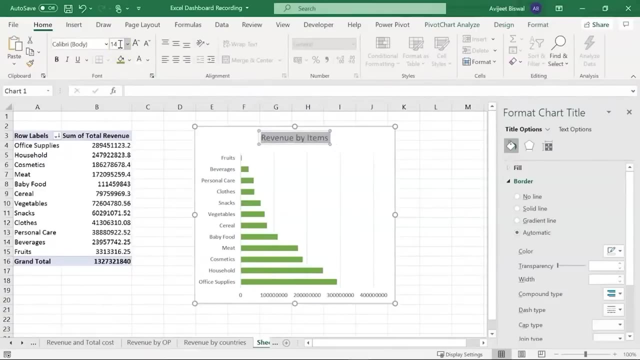 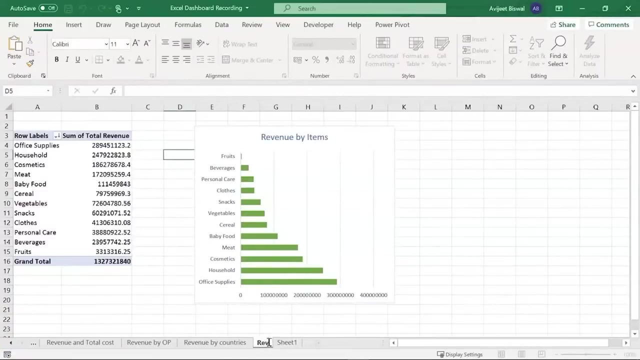 want to select green color? alright, i have edited my chart a bit now. let's make it 14 and i will remove the bold. ok, here, if you want, you can change the font also. let's keep it in blue color, alright. finally, let's rename this sheet, so i will write. 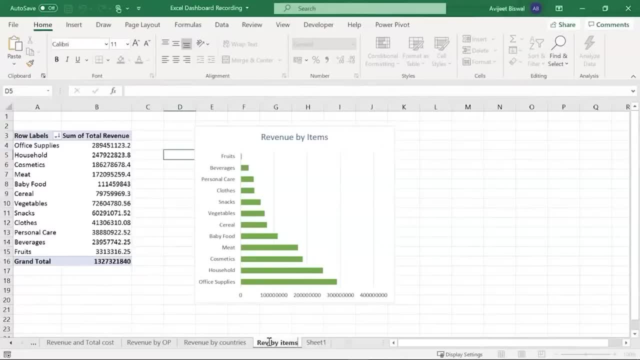 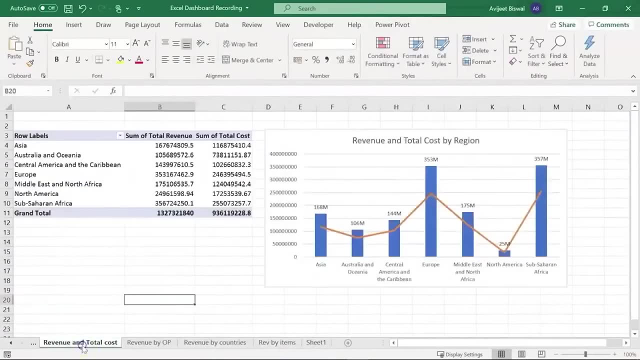 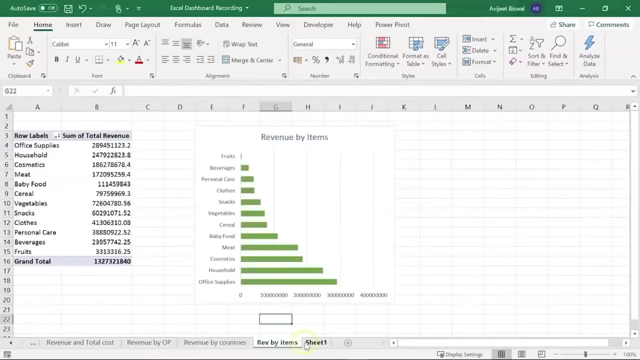 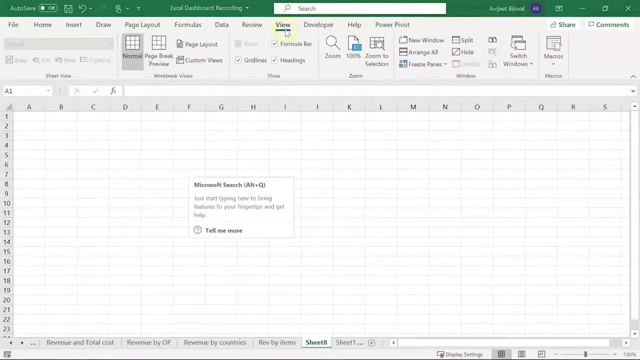 revenue by items- cool. finally. now it's time for us to merge all the charts that we have created to our dashboard, so let me show you how you can create the dashboard. i will create a new sheet and first thing i am going to do is i will click on the view tab. 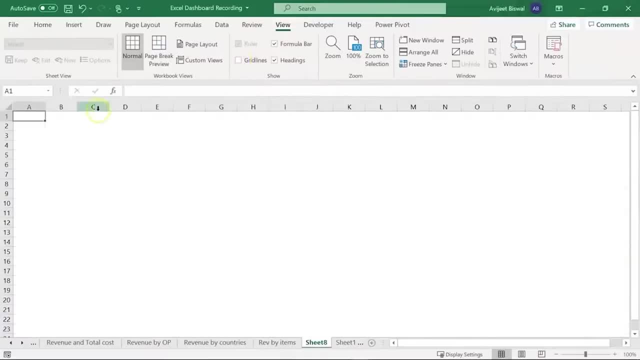 and uncheck grid lines. so this will remove the grid lines present in the worksheet. next, i am going to insert an image, so we will have a background image on our dashboard. so the way to do is i will go to the insert tab and under illustrations i have the option to select. 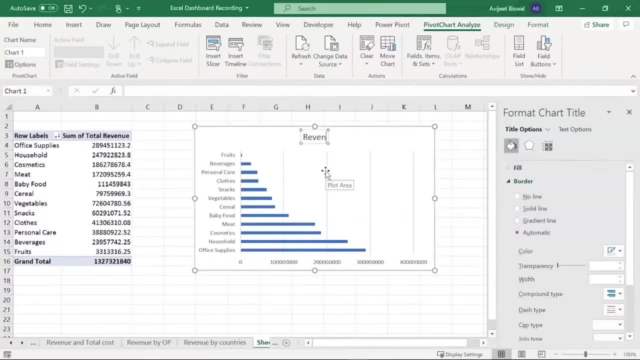 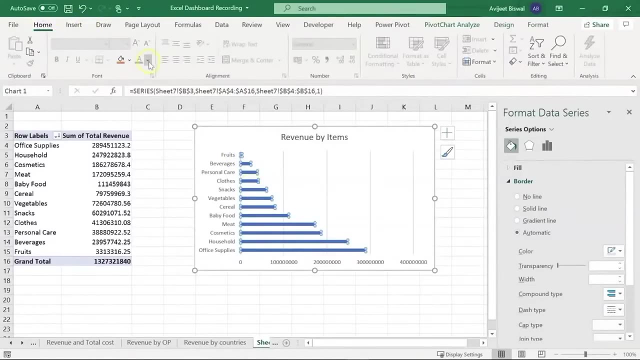 this is going to be revenue by items. cool, we also want to change the color of the bars. so I have selected all the bars. I'll go to my home tab and here let's say I'm going to select green color. alright, I've edited my chart a bit. now let's 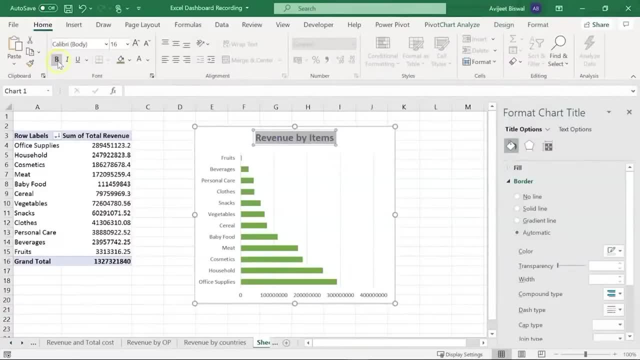 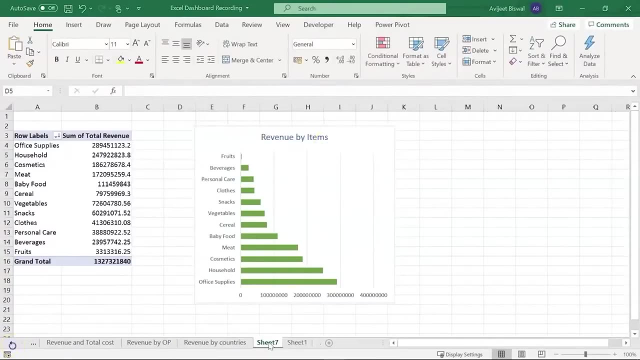 make it 14 and I'll remove the bold. okay, here, if you want, you can change the font. also, let's keep it in blue color, all right? finally, let's rename this sheet so I'll write revenue by items. cool, finally, now it's time for us to 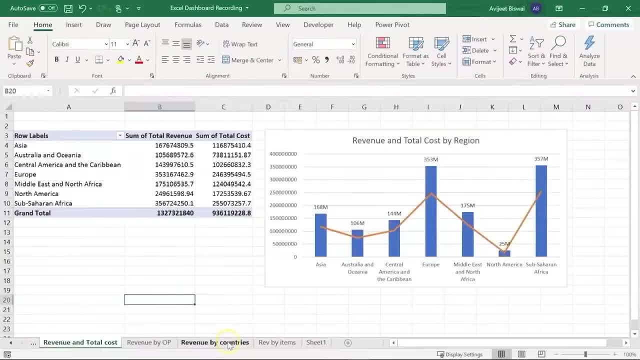 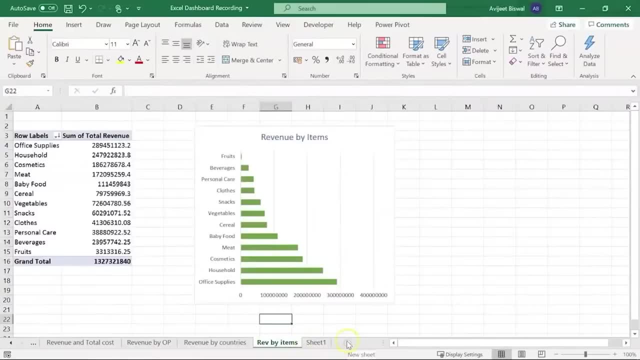 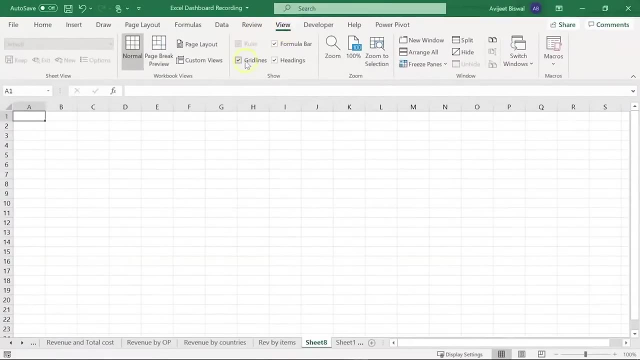 merge all the charts that we have created to our dashboard. so let me show you how you can create the dashboard. I'll create a new sheet and first thing I'm going to do is I click on the View tab and uncheck grid lines. so this will. 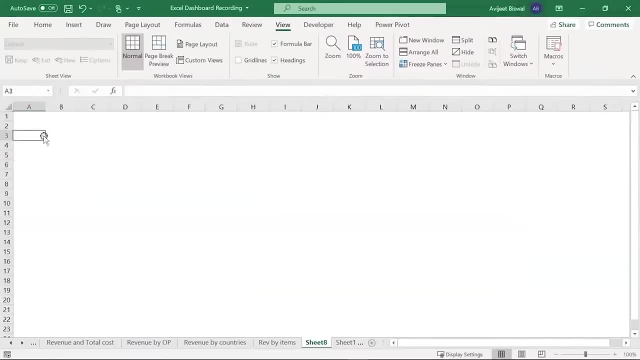 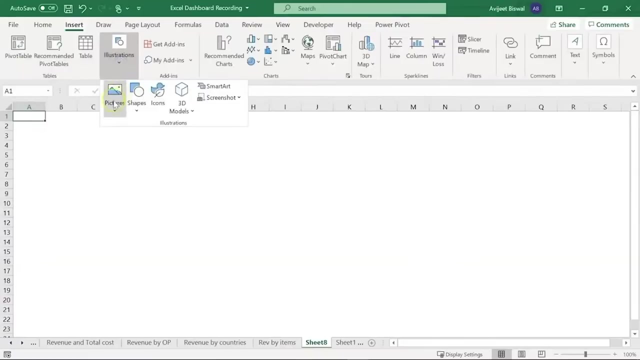 remove the grid lines present in the worksheet. next, I'm going to insert an image, so we'll have a background image on our dashboard. so the way to do is I will go to the insert tab and under illustrations I have the option to select pictures or insert pictures. so I'm going to insert picture. 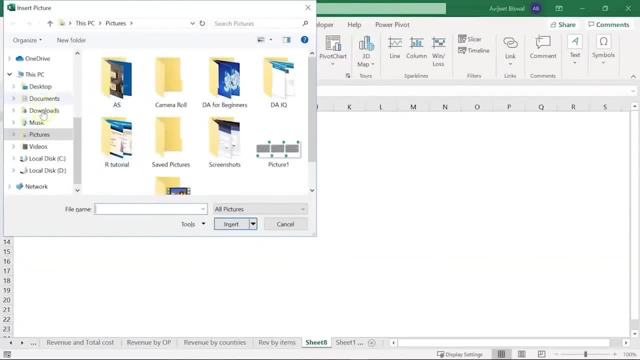 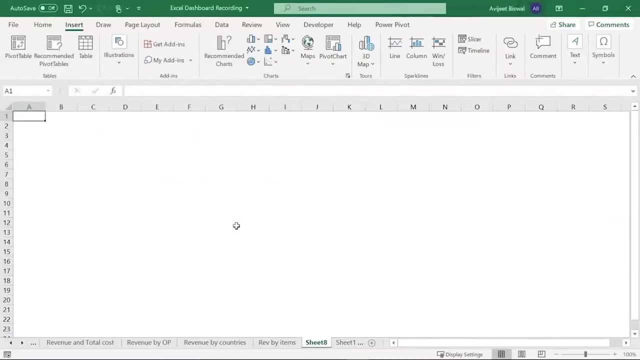 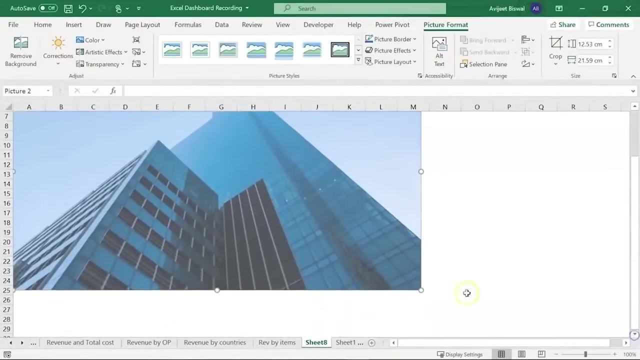 present on the device that is my computer. I'll go to desktop and here I have a folder called Excel dashboard files and I'll select this dashboard background and hit insert. so this is going to insert an image. now let me just drag this image. so it covers a fair enough portion. so I'll hit. 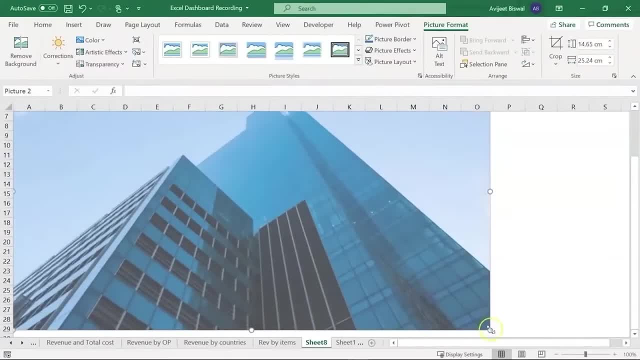 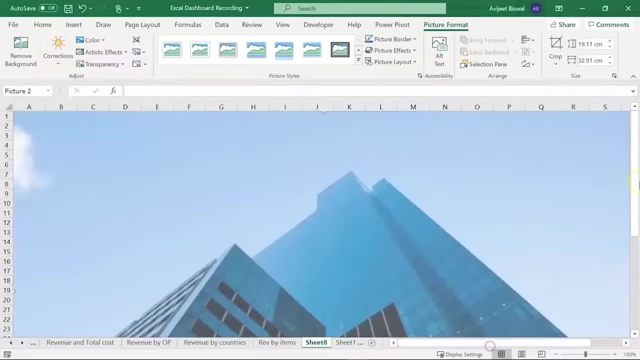 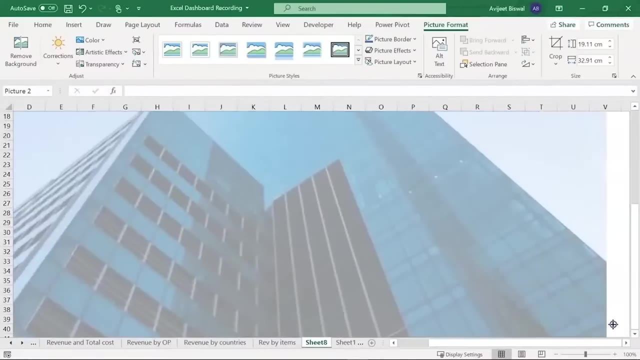 enter and it will show me the image. so I'll hit enter and it will show me the image. so I'll hit shift and I'll drag it all right. so you can see I have successfully added a background image. if you want, you can still expand this background image a bit. 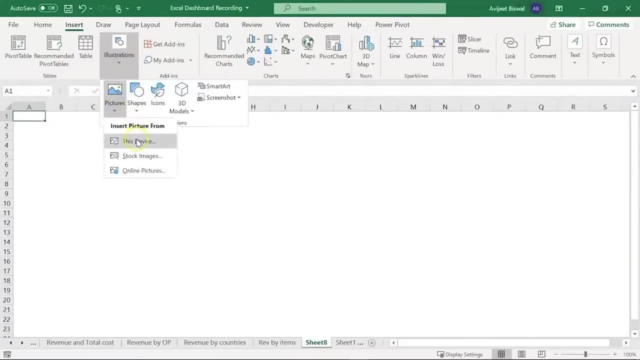 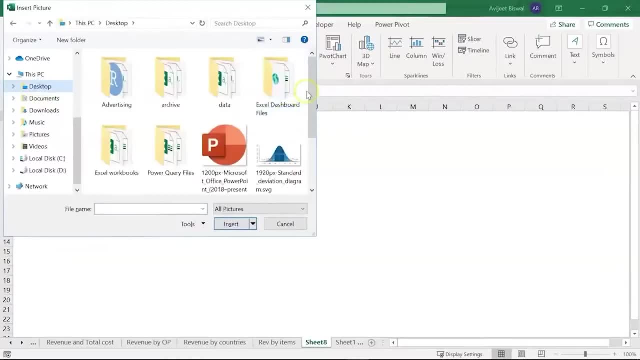 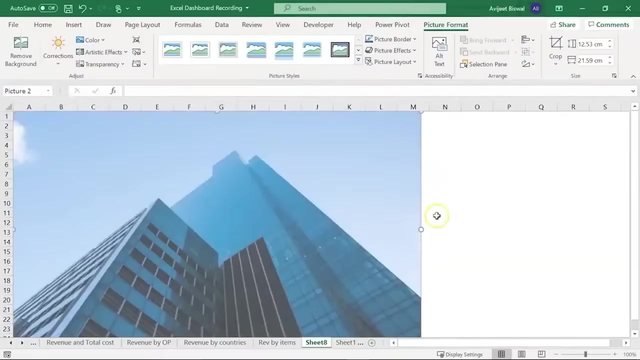 pictures or insert pictures. so i am going to insert picture present on the device that is my computer. i will go to desktop and here i have a folder called excel dashboard files and i will select this dashboard background and hit insert. so this is going to insert an image now. 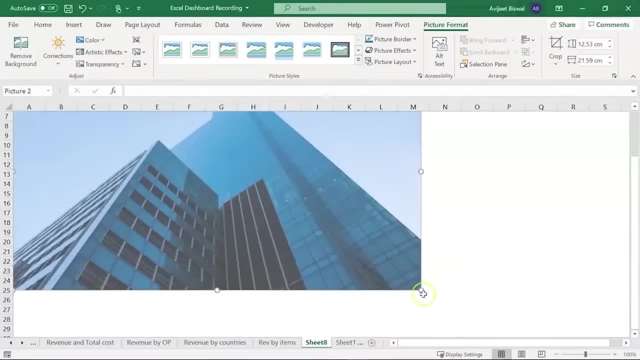 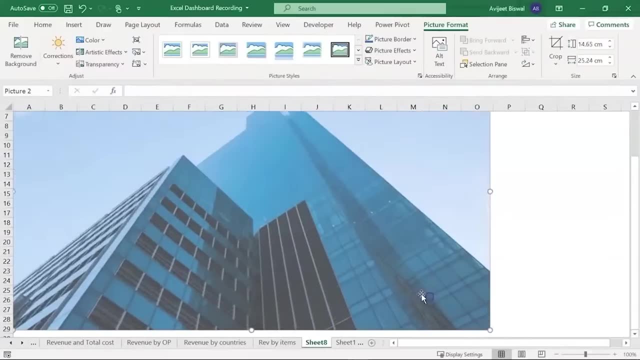 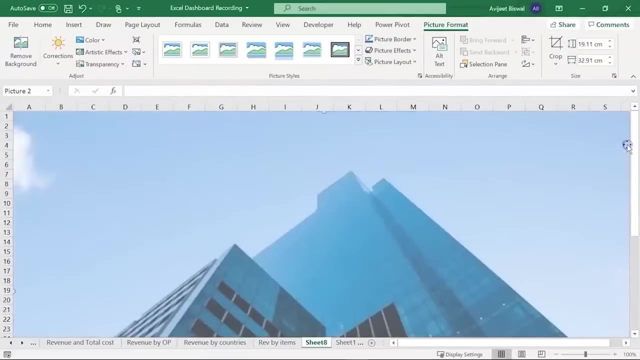 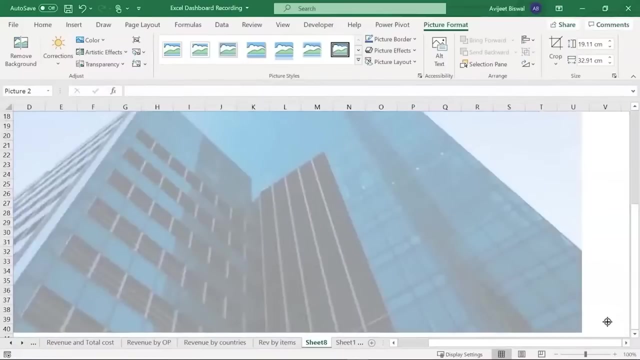 let me just drag this image so it covers a fair enough portion. so i will hit shift and i will drag it. alright, so you can see i have successfully added a background image. if you want, you can still expand this background image a bit to the right, cool. 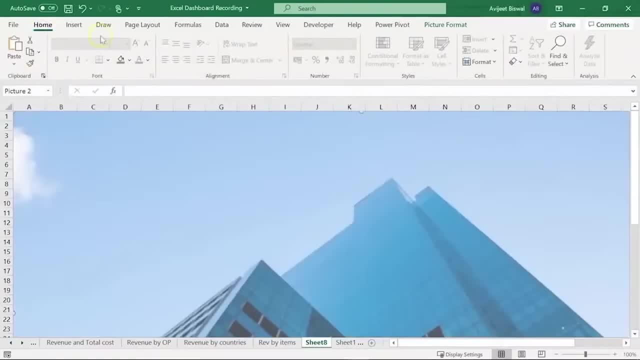 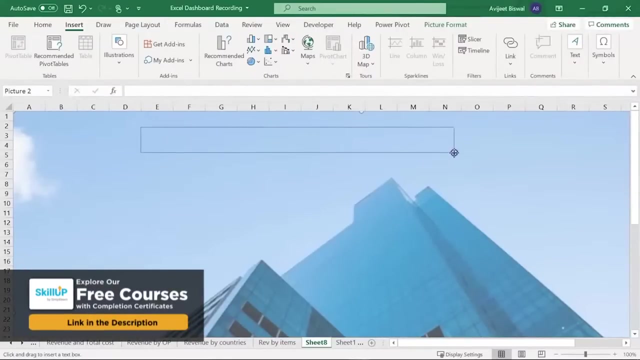 now the next thing is going to be the title of the dashboard. so i will click on insert and here i have the option to select a text box. so i will click on a text box and i am going to place a text box in the middle and i am going to name: 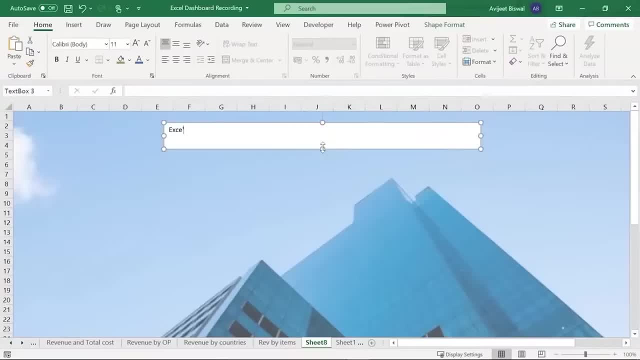 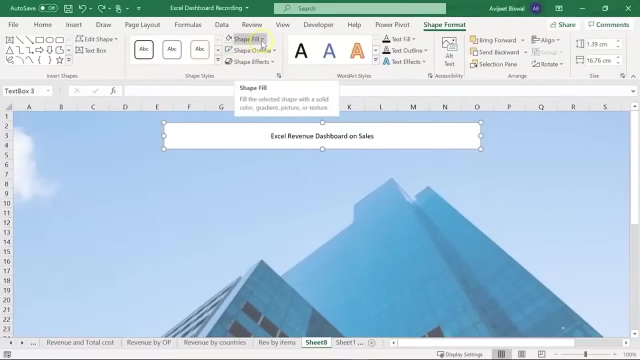 this text box as excel revenue dashboard on sales. i will central line it. lets do some more formatting, so i will select this text box on the top. you can see shape format here. i am going to expand this shape fill and i will select no fill. so my text box is transparent. 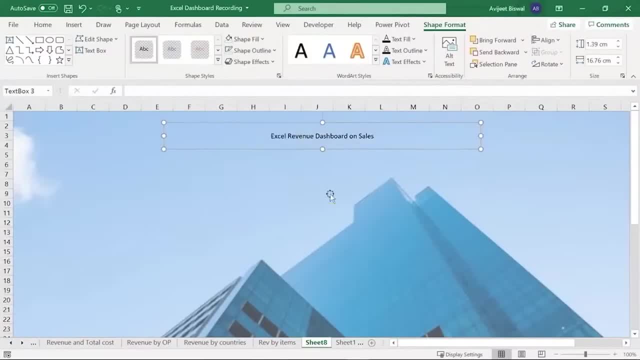 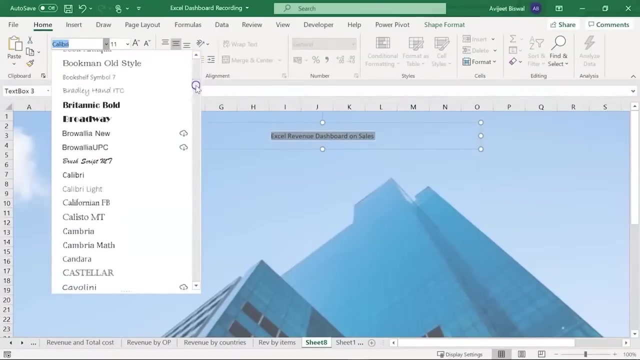 now, and i will also remove the outline. alright, now let me just double click on the title of my dashboard and i am going to select a font. you can select whichever font you want. let me stick to britannica bold and i will increase the size to, lets say, 30. 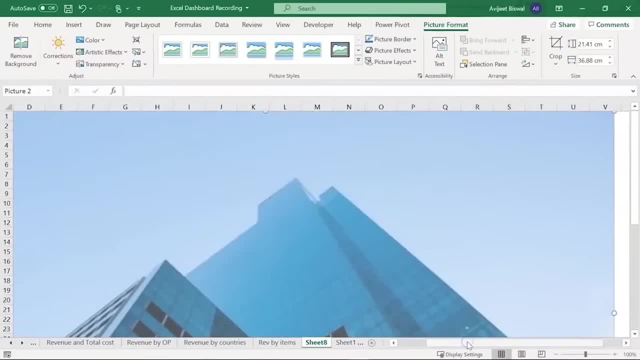 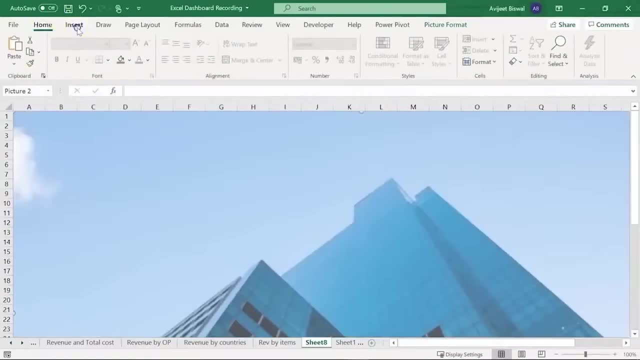 to the right. cool now. the next thing is going to be the title of the dashboard. so I'll click on the title of the dashboard. so I'll click on the title of the dashboard, so I'll click on insert, and here I have the option to select a. 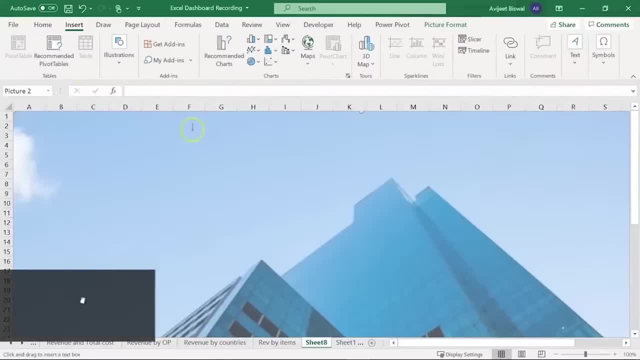 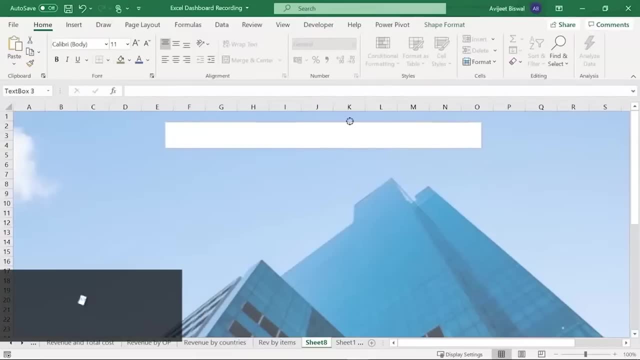 text box. so I'll click on a text box and I'm going to place a text box in the middle and I'm going to name this text box as Excel revenue dashboard on sales. I'll central line it. let's do some more formatting, so I'll select this. 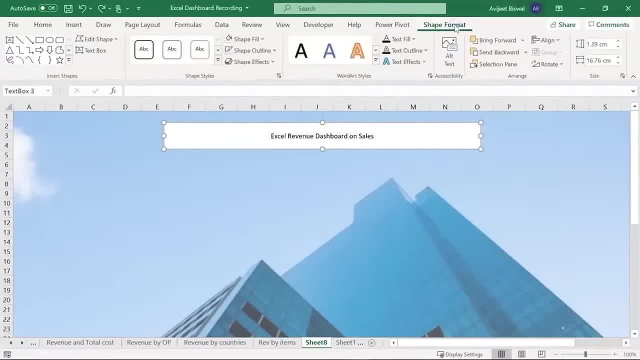 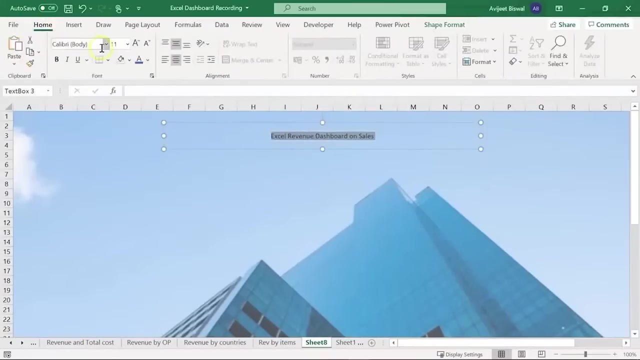 text box on the top. you can see shape format here. I'm going to expand this shape fill and I'll select no fill. so my text box is transparent now and I'll also remove all the outline. all right now let me just double click on the title of my dashboard and I'm going to 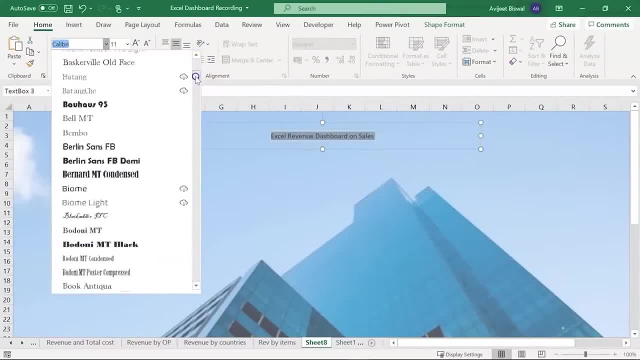 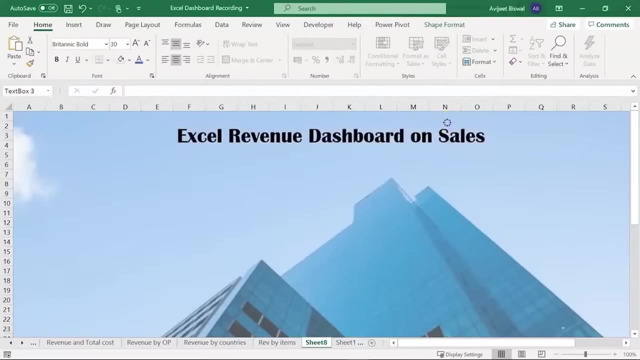 select a font. you can select whichever font you want. let me stick to Britannica bold and I'll increase the size to, let's say, 30. all right, I'll just drag the text box. I'll make the text, as my, white instead of black. all right? so we have our title of the dashboard ready now, if you want you. 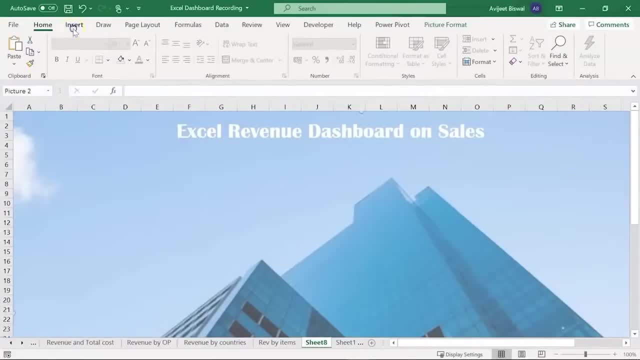 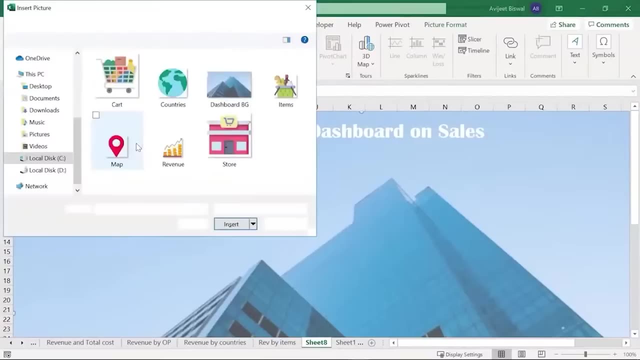 can also insert some icons to this dashboard, so I'll go to insert and I'll click on illustrations again and select pictures. I'm going to add this to pictures which is of a store and a cart to make it look like a picture of a store and a cart. I'm going to add this to pictures which is of a store. 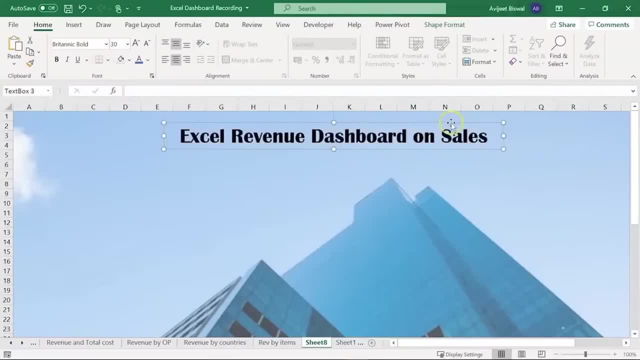 alright, i will just drag the text box. i will make the text as white instead of black. alright, so we have our title of the dashboard ready now. if you want, you can also insert some icons to this dashboard. so i will go to insert and i will click on. 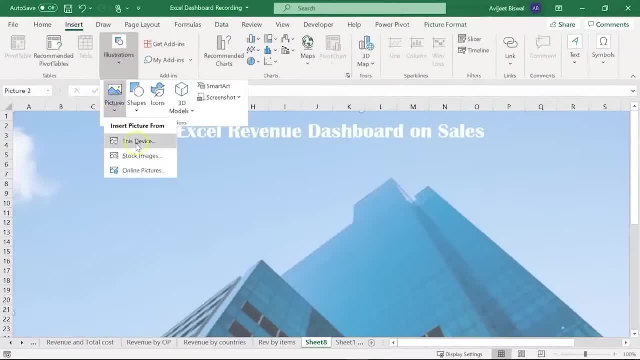 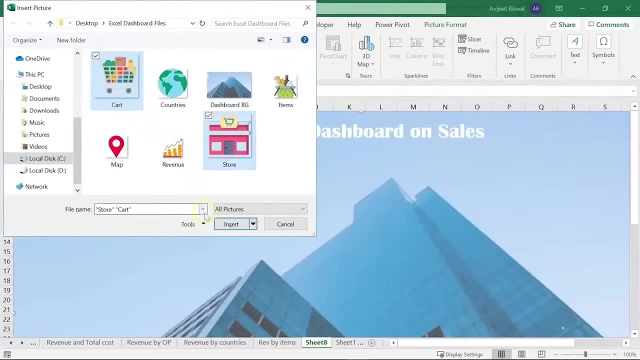 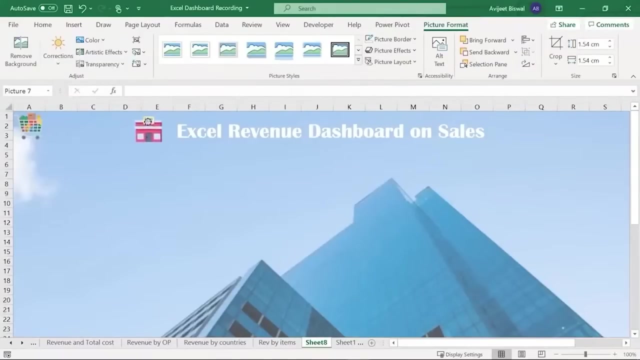 illustrations again and select pictures. i am going to add this, two pictures, which is of a store and a cart, to make it look visually appealing. so i will place the icons here and similarly, let me just copy it and i will place the cart and the store to the right as well. 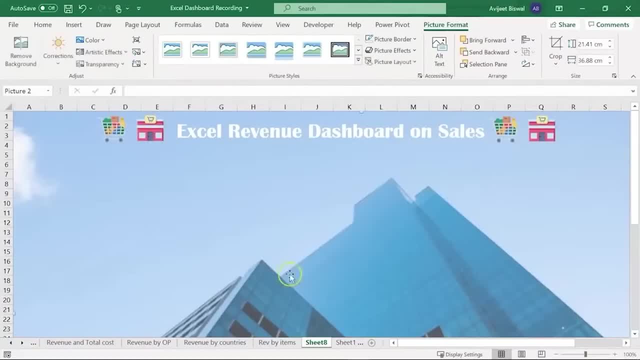 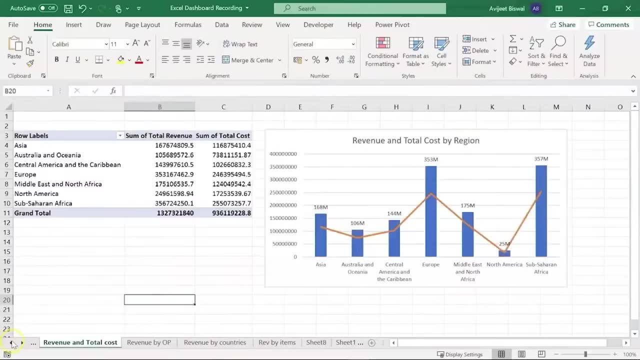 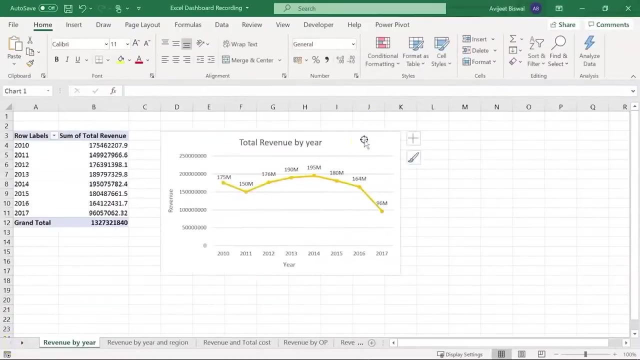 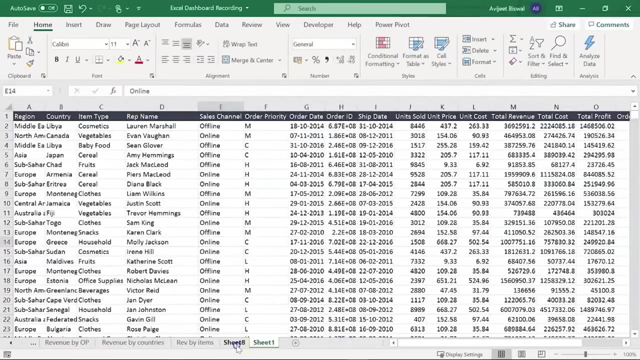 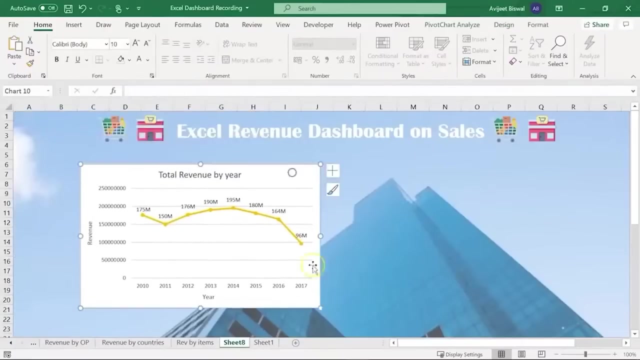 alright. next, the idea is to bring in all the charts that we have created and place it on the dashboard. so let me copy each of the charts and place it on the dashboard. so i will hit control v to paste it and we will resize this as well. 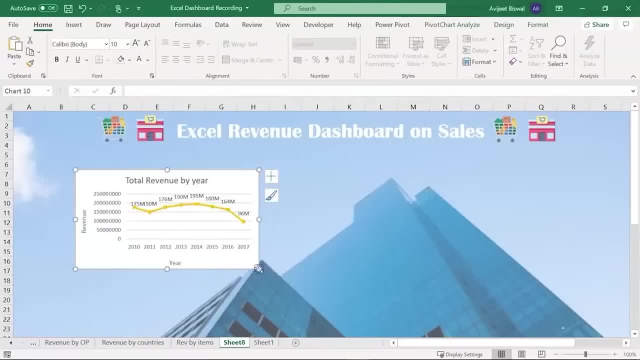 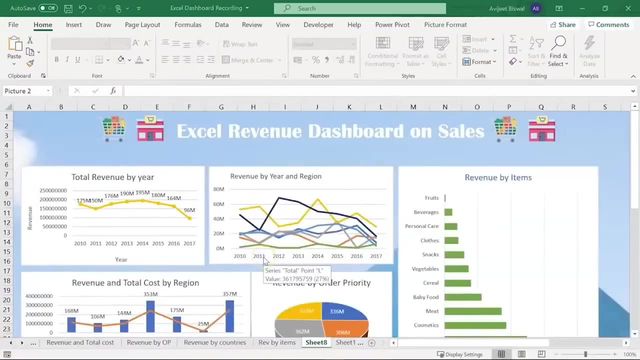 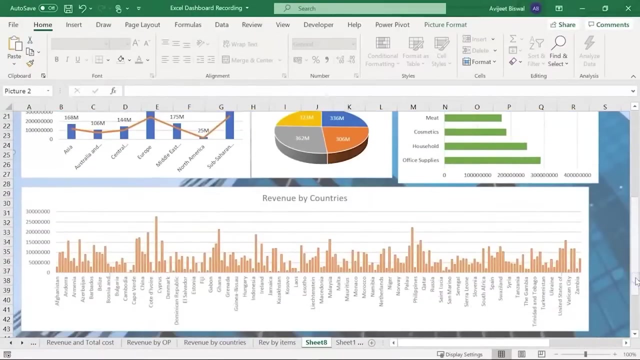 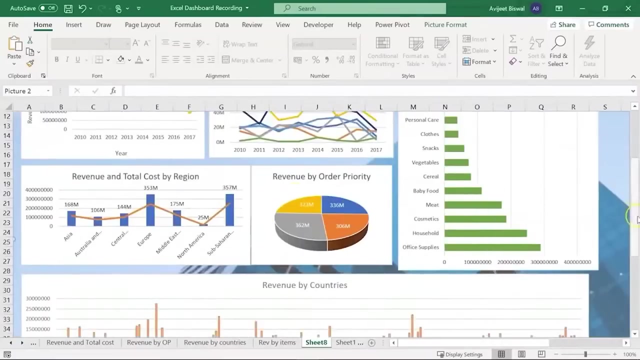 alright. similarly, let me bring in all the other charts as well. alright, so now you can see. i have added all my charts and graphs to this dashboard, so you can see. here we have our line charts, our column charts, the combo charts, the spy chart and others. now let me go. 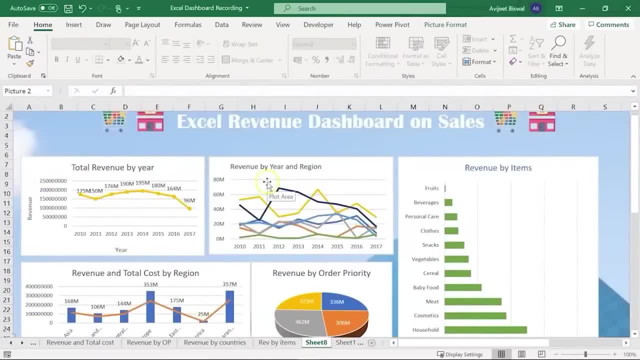 ahead and format these charts a little more, so you can see this looks a bit cluttered. so let's adjust the labels. let me bring this down. similarly, i will bring 190 million a little below. alright, this looks fine. now. one more thing we are going to do is 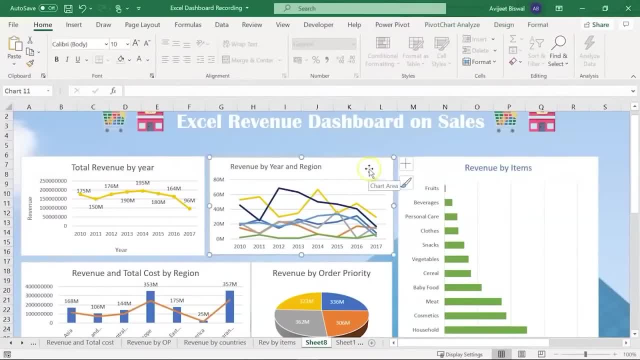 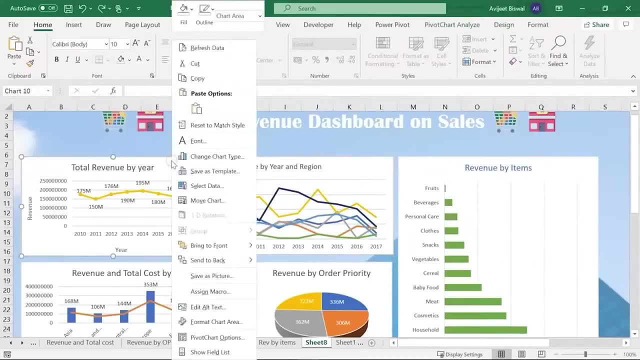 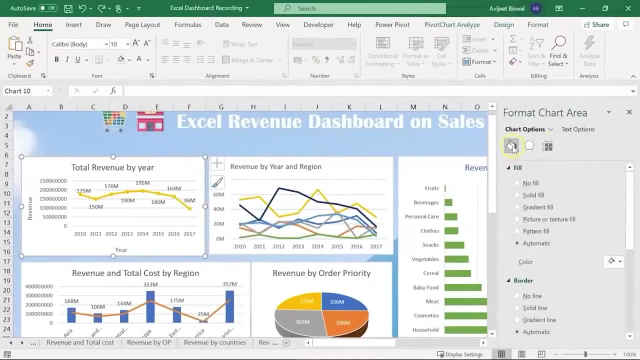 we will remove the white background from each of the charts and make it transparent. so let me show you how to do it. so i will select this chart, then i will right click and go to format chart area. here on the right you see, we have an option called no fill. 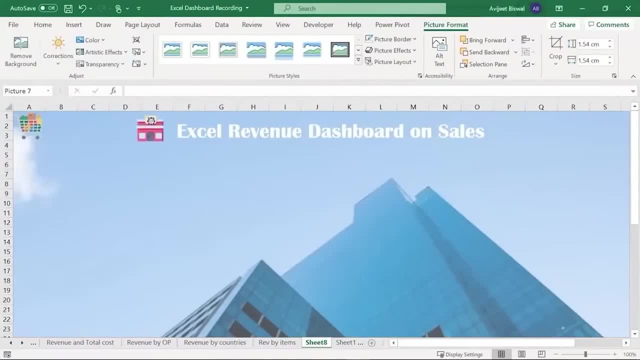 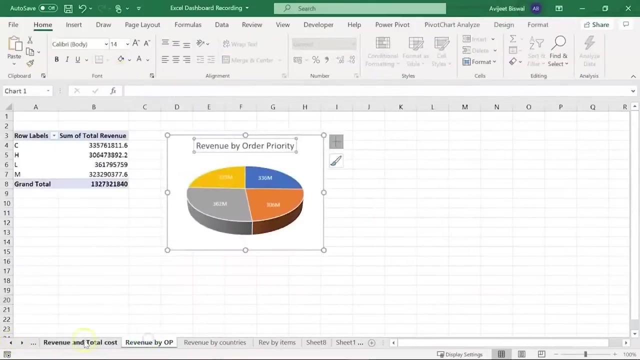 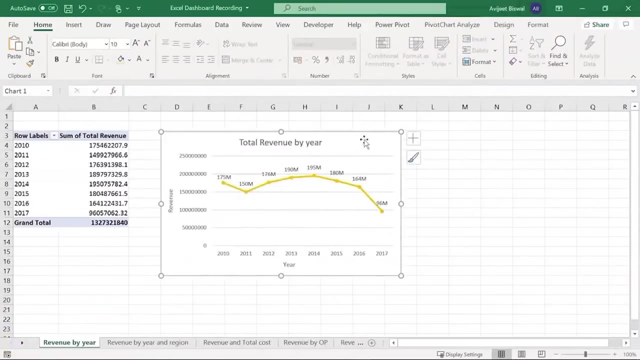 visually appealing, so I'll please the icons here and, similarly, let me just copy it and I'll place the cart and the store to the right as well. alright, next, the idea is to bring in all the charts that we have created and place it on the dashboard. so let me copy each of the charts and place it. 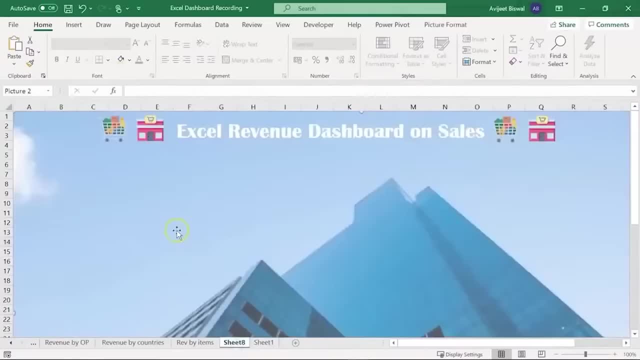 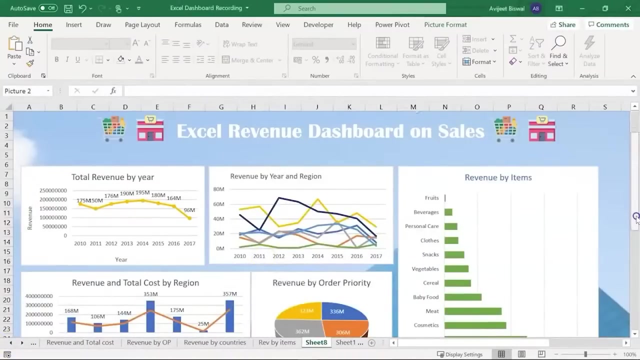 on the dashboard, so I'll hit control V to paste it and we'll resize this as well, all right? similarly, let me bring in all the other charts as well. all right, so now you can see. I have added all my charts and graphs to this dashboard, so 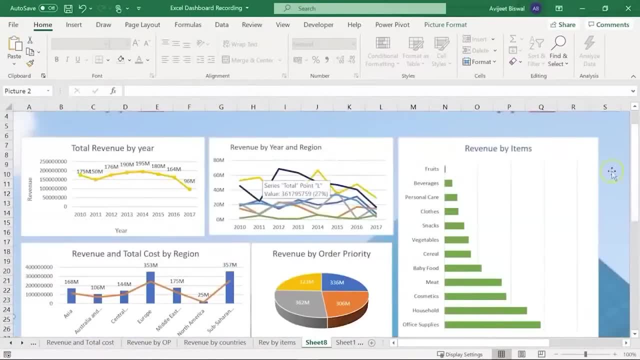 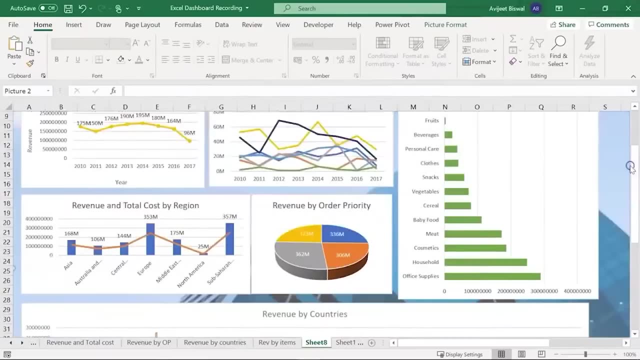 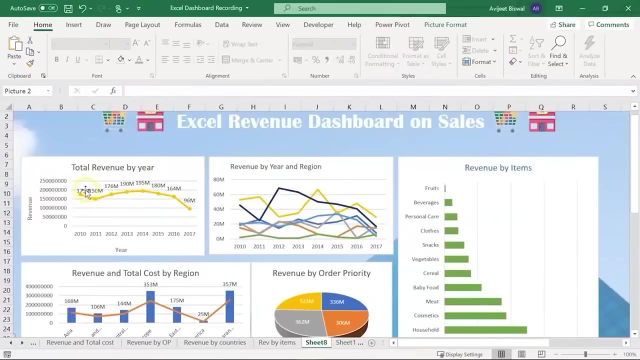 you can see, here we have our line charts, our column charts, the combo charts, the spy chart and others. now let me go ahead and format these charts a little more so you can see this looks a bit cluttered, so let's adjust the labels. let me bring 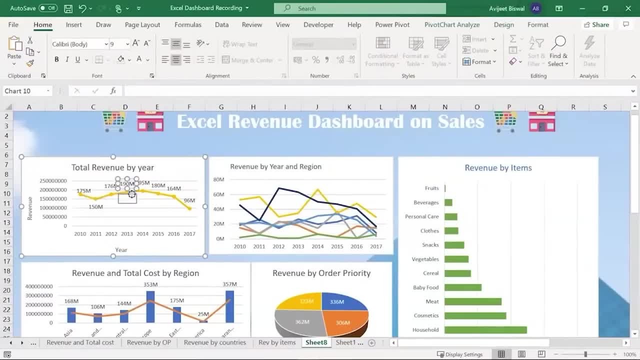 this down. similarly, I'll bring 190 million a little below you. all. right, this looks fine. now one more thing we are going to do is we'll remove the white background from each of the charts and make it transparent. so let me show you how to do it. so I'll select this chart, then I'll right click and go. 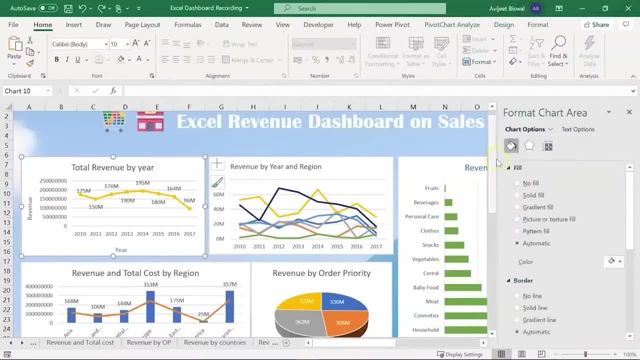 to format chart area. here on the right. you see we have an option called no fill. so if I select no fill, you can see the white background is gone now. similarly, let me also remove the grid lines. so I'll select the grid lines and hit delete. so I've also removed the grid lines from here. 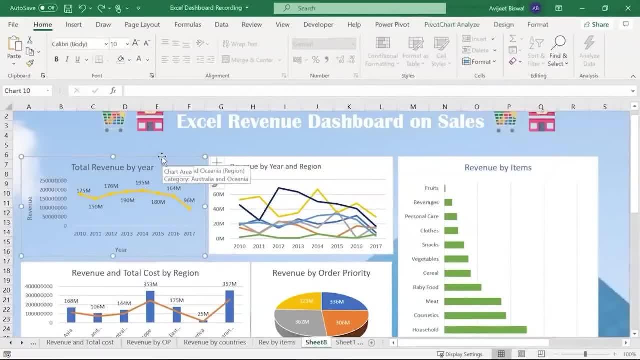 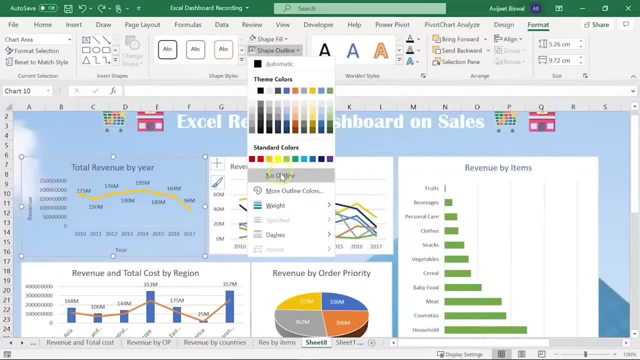 now let's also remove the white outline that we have. so I'll select this chart, go to format and here I'll go to shape outline and I'll select no outline. you see this, so we have our total revenue by year, which is a line chart, and this is: 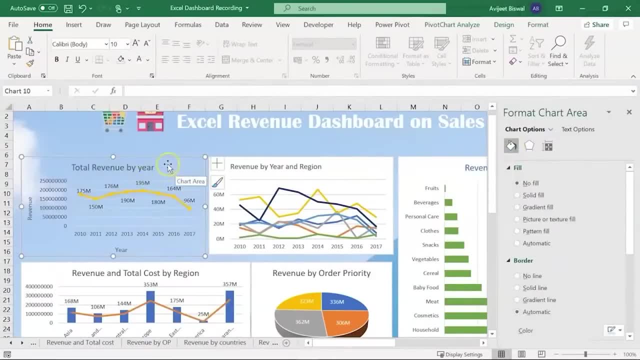 so if i select no fill, you can see the white background is gone now. similarly, let me also remove the grid lines, so i will select the grid lines and hit delete. so we have also removed the grid lines from here. now let's also remove the white outline that we have, so i will select. 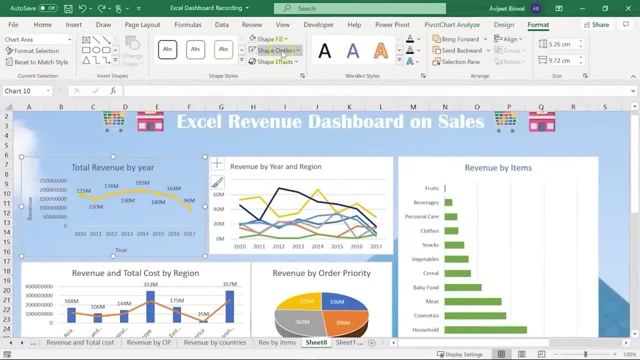 this chart, go to format, and here i will go to shape outline and i will select no outline. you see this? so we have our total revenue by year, which is a line chart, and this is completely transparent now. now, what i am going to do is i will place this chart. 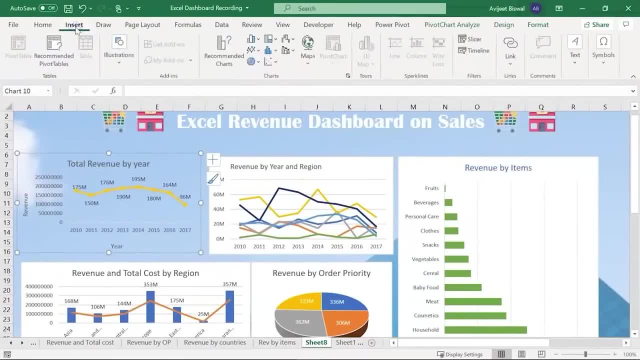 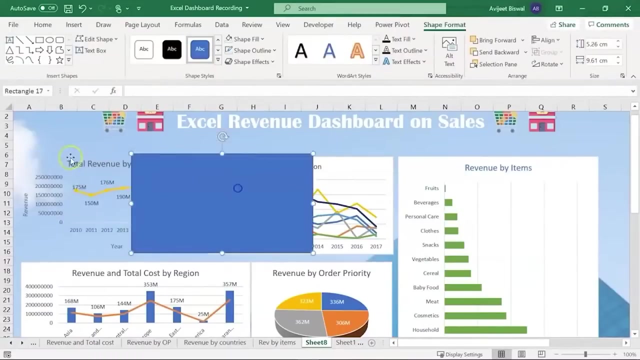 over a box. so i will go to insert and in insert we have the option to create a shape. so i will click on illustrations and here i will choose a shape and let me select a rectangle. so i will just create a rectangle here. alright, and now what i will do is: 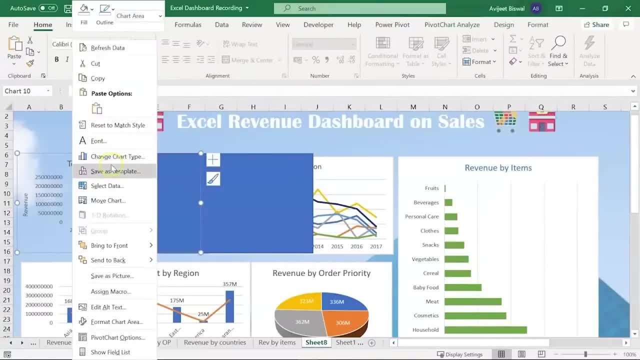 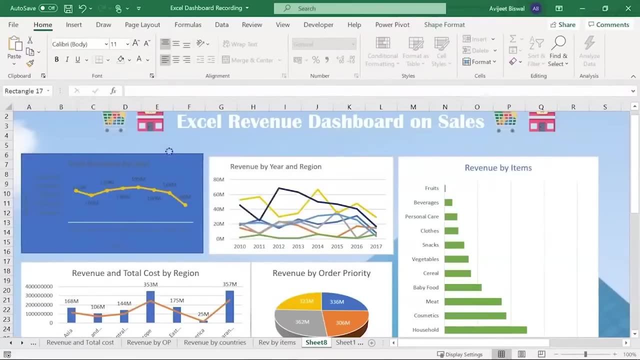 i will select this and bring this to front. i will right click and choose, bring to front, and i will place this shape below it. alright, now the next thing is to edit the shape. so first i will change the color of this box. so let me select this. 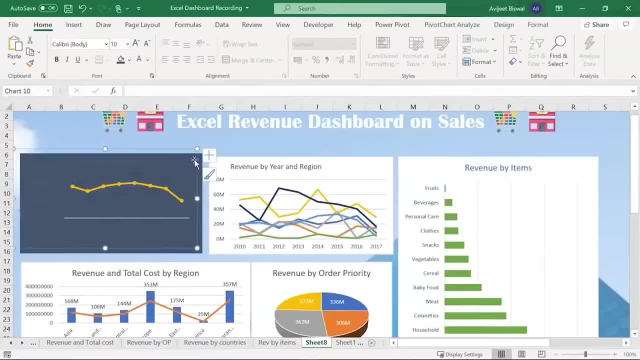 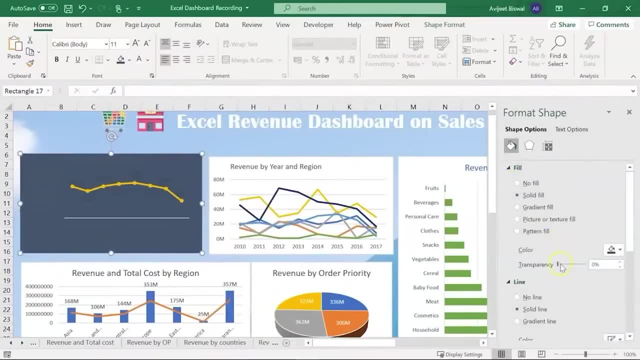 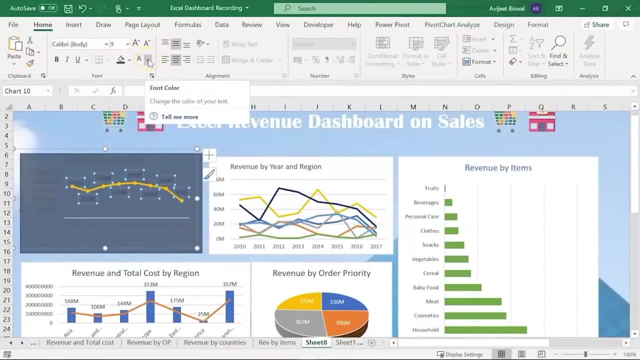 blue color and let me increase the transparency. so i will right click and go to format shape here i will increase the transparency. let's keep it to 25%, or let's say 20%. alright, next thing, we will just convert all the font to white. 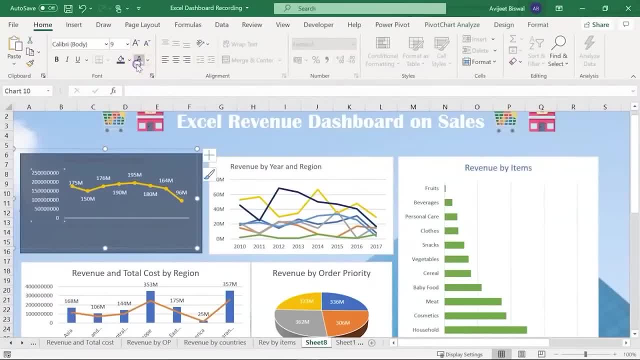 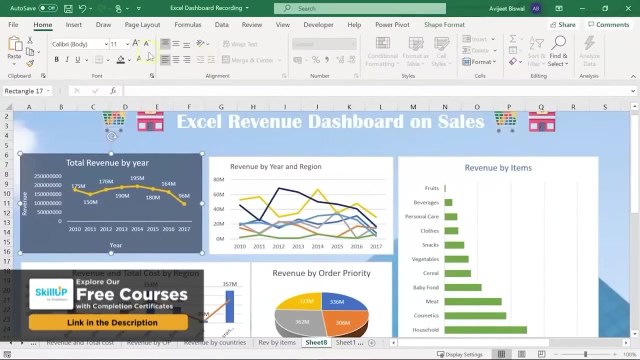 color, including the axis labels, the chart title. we will also convert all the axis labels to white color so it looks better now we will just adjust our chart over here. next thing: let's just remove the outline. so i will go to shape outline and i will select no outline. 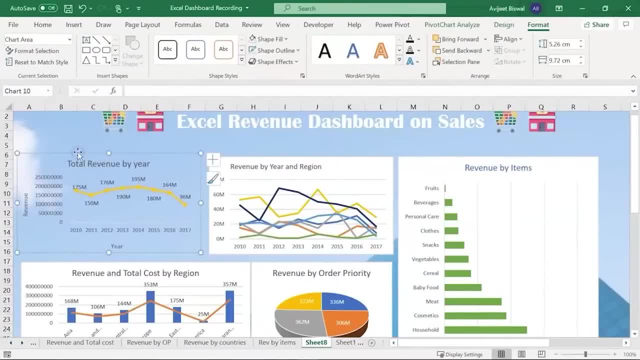 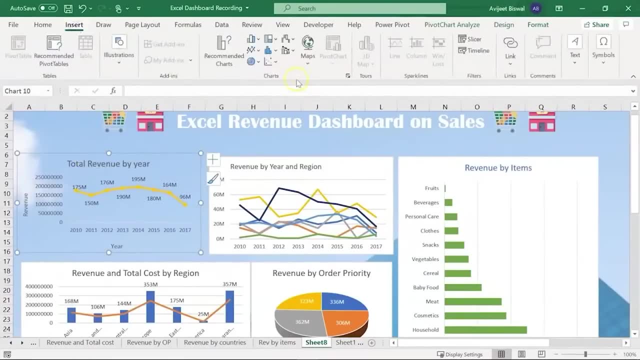 is completely transparent now. now what I'm going to do is I'll place this chart over a box, so I'll go to insert, and in insert we have the option to create a shape. so I'll click on illustrations and here I'll choose a shape and let me select a rectangle. so I'll just create a rectangle here. 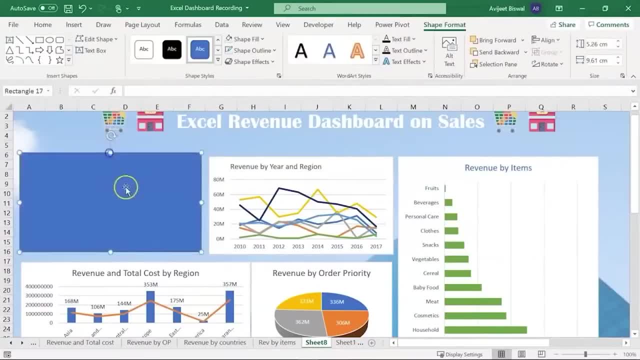 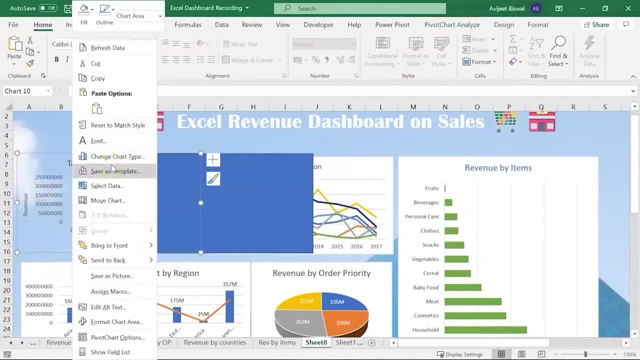 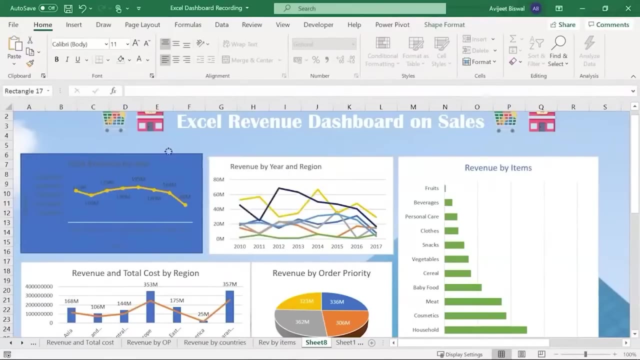 all right, and now what I'll do is I'll select this and bring this to front. I'll right click and choose bring to front and I'll place this shape below it all. right now. the next thing is to edit the shape. so first I'll change the color of this. 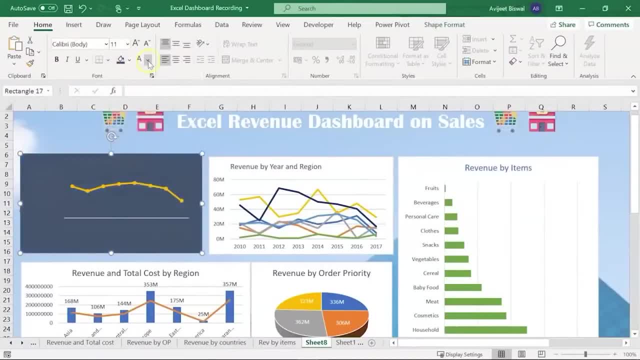 box. so let me select this blue color and let me increase the transparency. so I'll right click and go to format shape. here I'll increase the transparency. let's keep it to 25%, or let's say 20%. all right, next thing, we'll just convert. 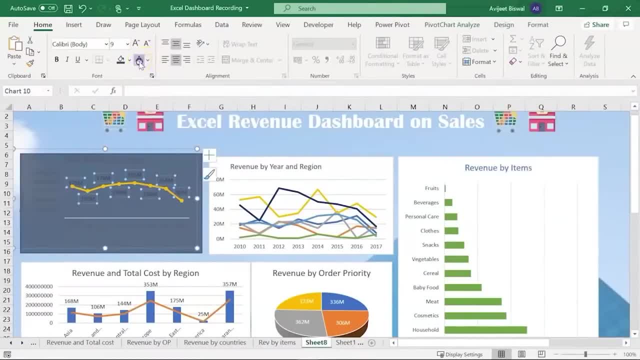 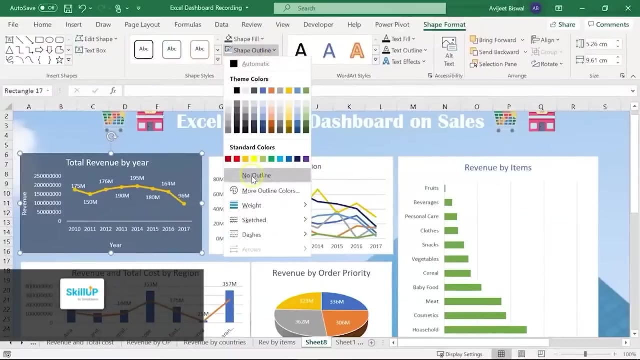 all the font to white color, including the axis labels, the chart title. we'll also convert all the axis labels to white color so it looks better now we'll just adjust our chart over here. next thing: let's just remove the outline. so I'll go to shape outline and I'll 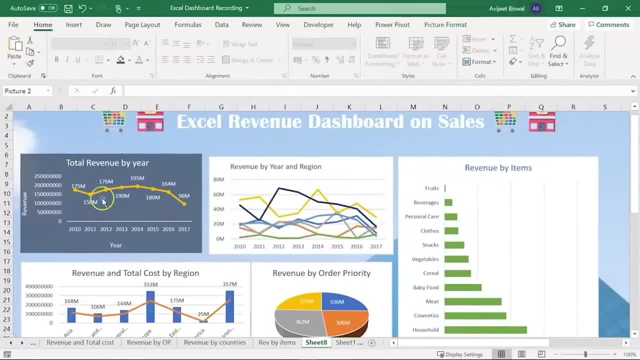 select no outline. you see, we have now formatted our chart. let's just pull the this a little up. all right now we'll add this blue background to all the other charts. so we'll first add the background, make it transparent, and then we'll convert the font text to white color. 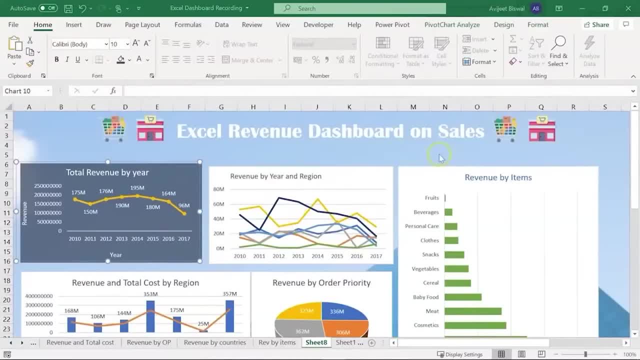 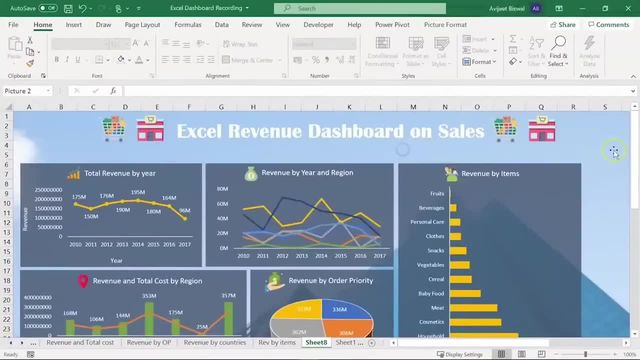 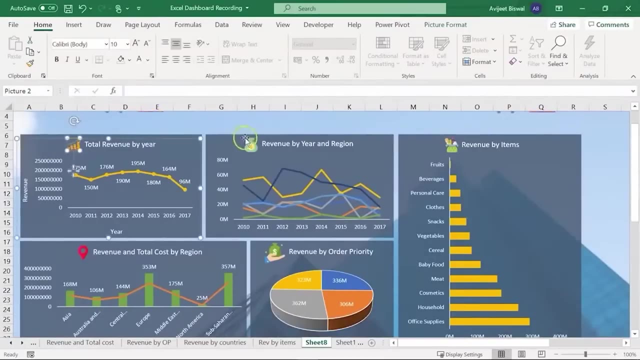 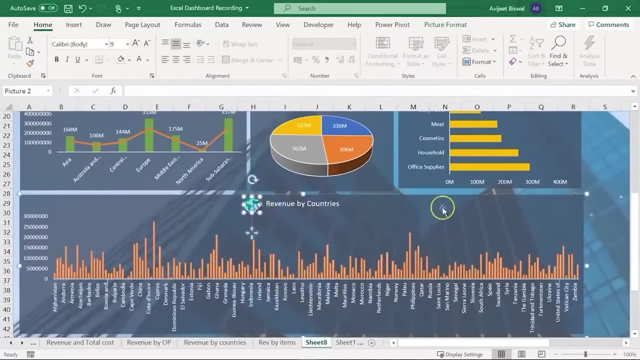 to make it more readable and visible. so for the time being I'll just pause the video and come back again. all right, so now you can see on your screens. we have nicely formatted our dashboard. so I've added a few logos for each of the charts. you can see the logos here. so for revenue by countries, we 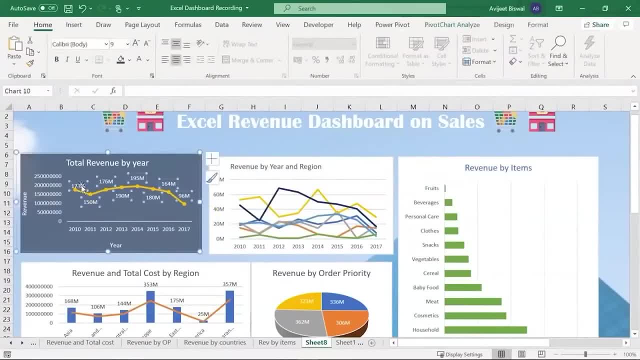 you see, we have now formatted our chart. let's just pull this a little up. alright, now we will add this blue background to all the other charts. so we will first add the background, make it transparent, and then we will convert the font text to white color to make it more readable. 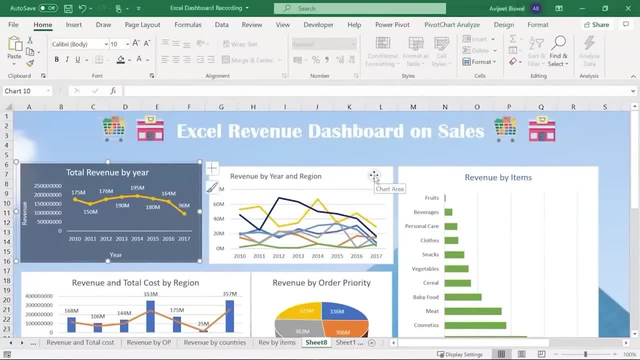 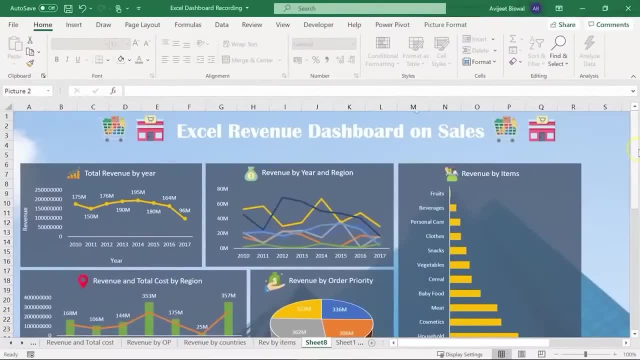 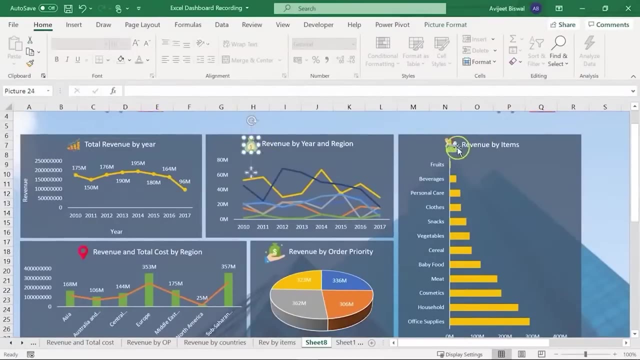 and visible. so for the time being i will just pause the video and come back again. alright, so now you can see on your screens. we have nicely formatted our dashboard so i have added a few logos for each of the charts. you can see the logos here. so for revenue by 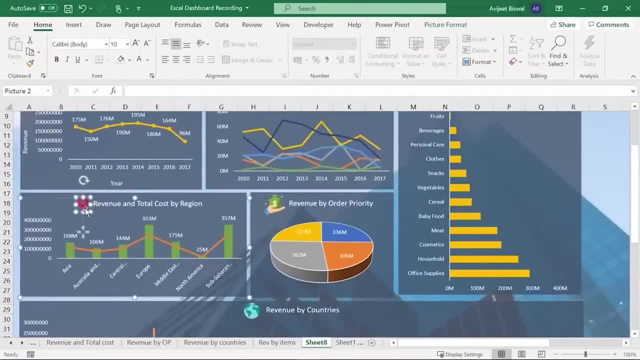 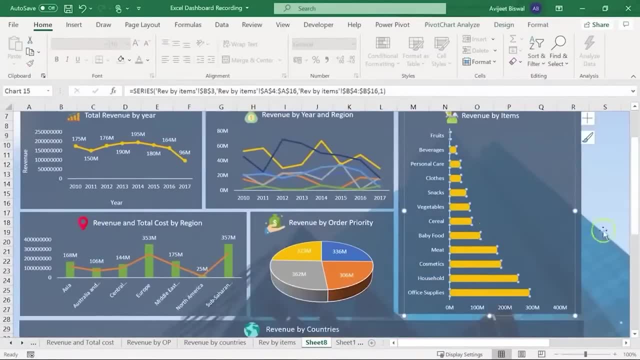 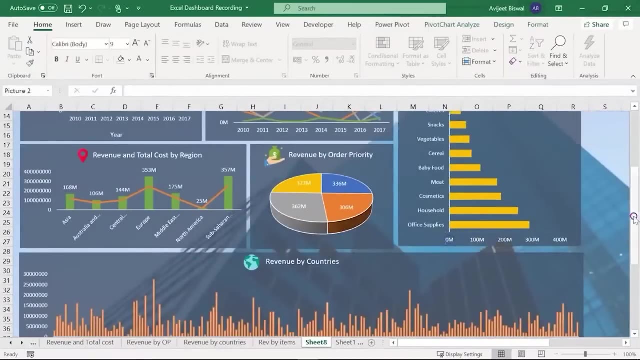 countries. we have a globe. then if you see here, this is kind of a map or a location. similarly, we have all formatted the color of the bars. then we have also formatted the labels in terms of millions. if you look on the y axis, even the revenue for year and region are all. 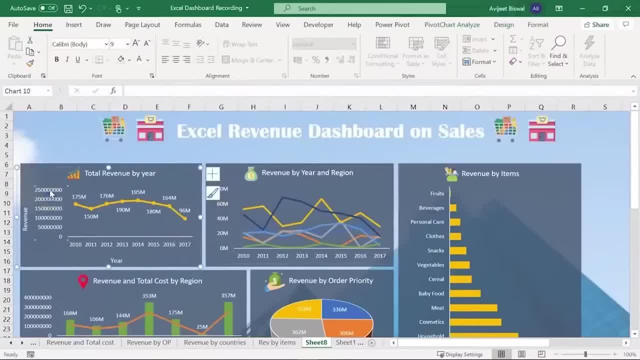 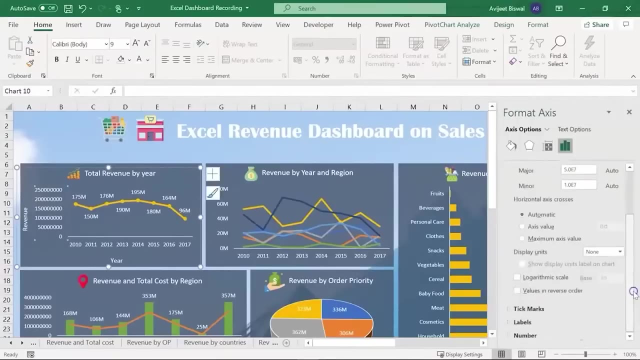 formatted in terms of millions. if you want this, you can also format the total year by revenue in terms of millions. so the way to do is you can select this graph, right click and go to format axis here. if i scroll down, you have numbers and under category, 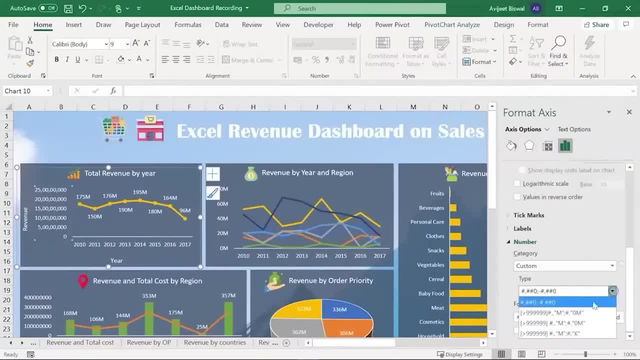 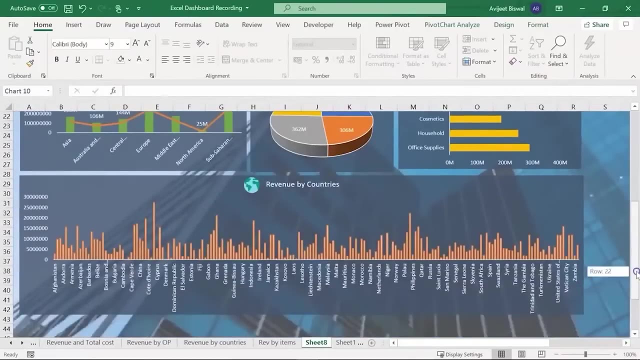 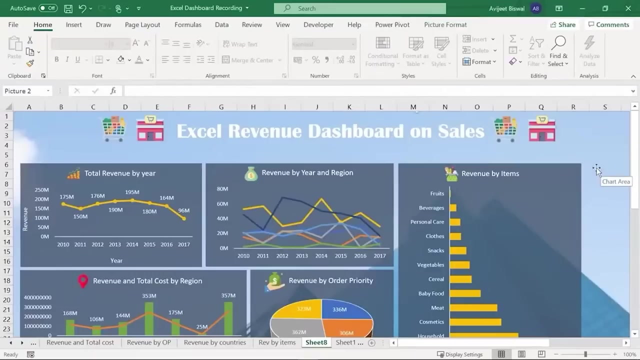 i will select custom, then i will select my type as this format, which is in millions. and you see, here we have successfully formatted our y axis labels. alright, so the next thing is to add slicers and timelines to our dashboard. now, slicers are used to format your data based on a particular 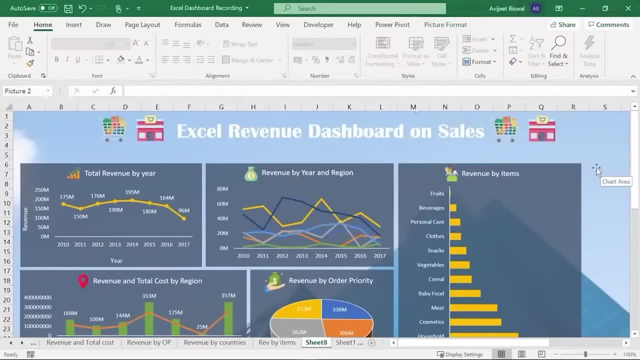 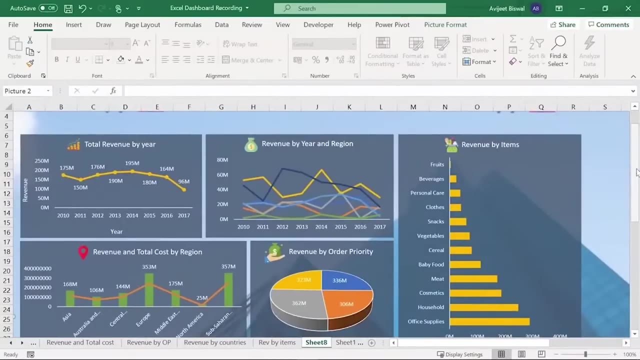 column. suppose if you want to see revenue by certain items, you can add item as a slicer and you can view the entire dashboard. similarly, for timelines you can add date columns. so if you want to see what was the amount of sales or revenue generated on a particular year or 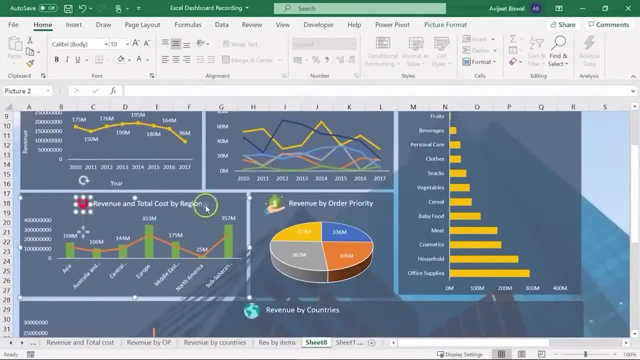 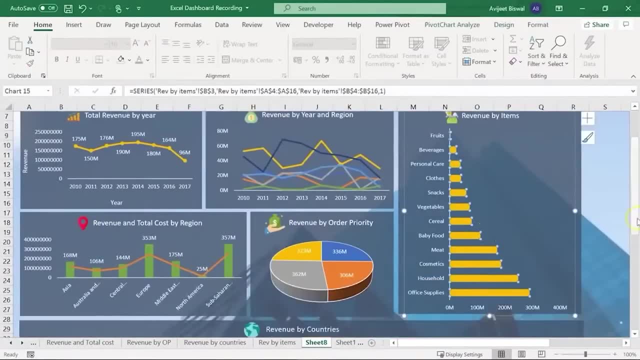 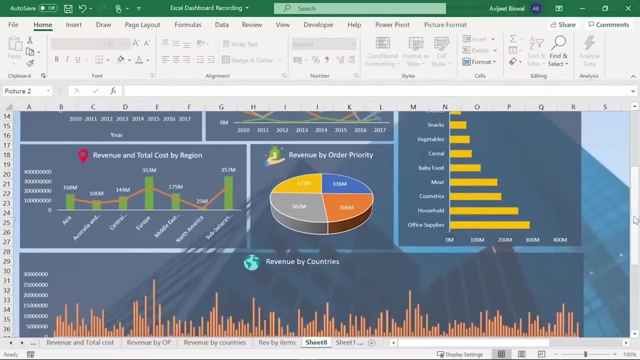 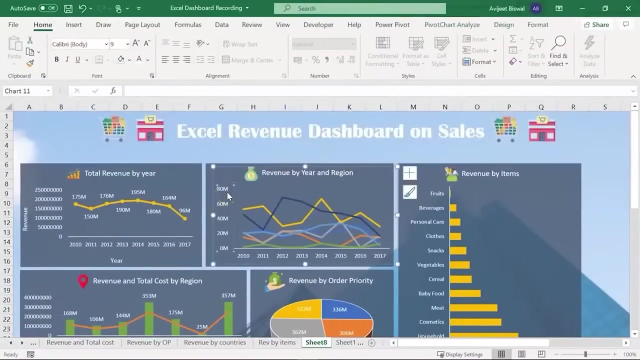 have a globe, then if you see here, this is kind of a map or a location. similarly, we have all formatted the color of the bars. then we have also formatted the labels in terms of millions. if you look on the y-axis, revenue for year in region are all formatted in terms of millions. 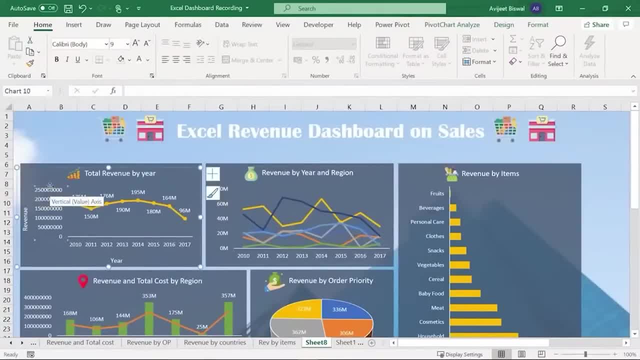 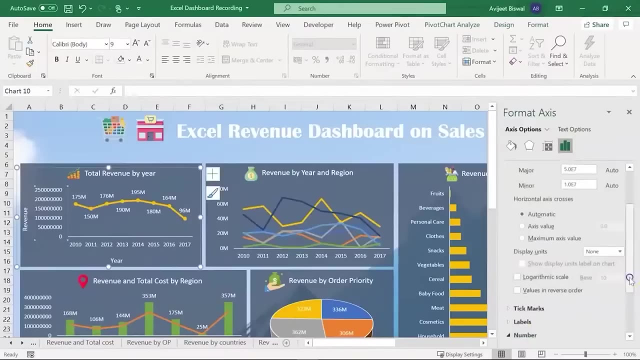 if you want this, you can also format the total year by revenue in terms of millions. so the way to do is you can select this graph, right click and go to format access here, if I scroll down, you have numbers and under category I'll select custom. then I'll select my type as. 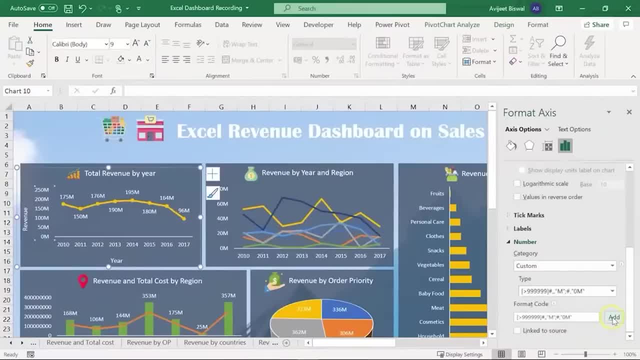 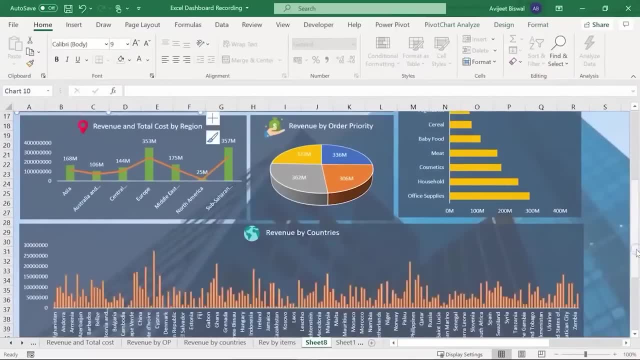 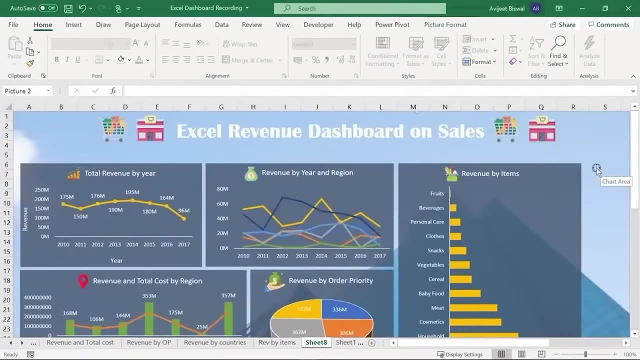 this format, which is in millions. and you see, here we have successfully formatted our Y axis labels. all right, so the next thing is to add slicers and timelines to our dashboard. now, slicers are used to format your data based on a particular column, suppose if you want to see revenue by certain. 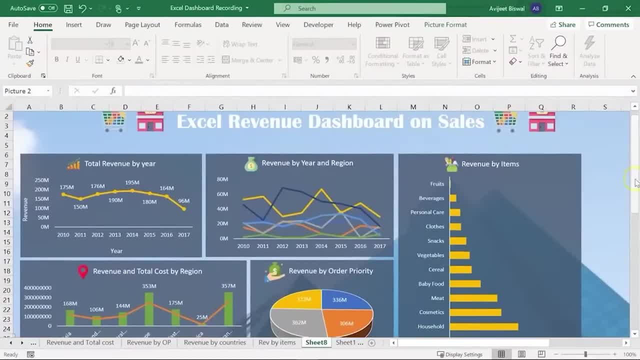 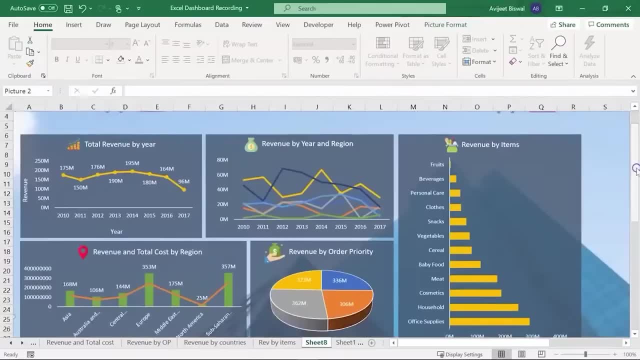 items. you can add item as a slicer and you can view the entire dashboard. Similarly, for timelines, you can add date columns. so if you want to see what was the amount of sales or revenue generated on a particular year or a particular month, you can do that. 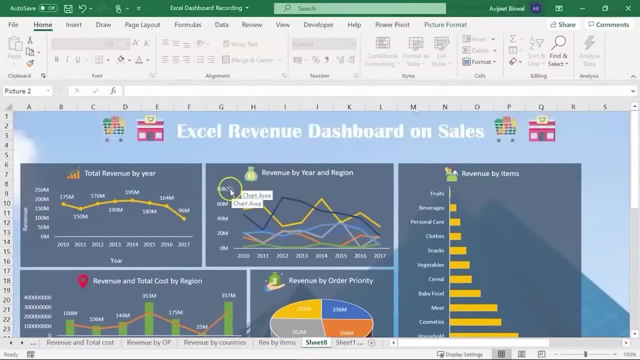 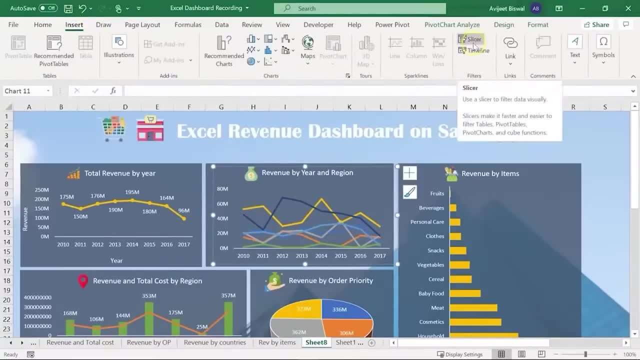 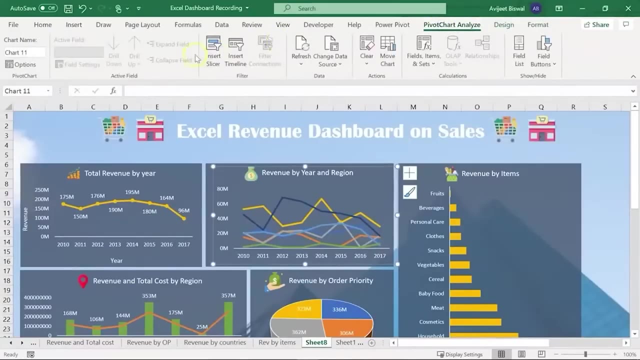 using a timeline. So I'll select one of the charts and then either you can go to the insert tab- and here you can see under filters we have slices and timeline- or if you go to the pivot chart analyze tab, here also you have insert slicer and timeline option. so I'll select insert slicer here first. 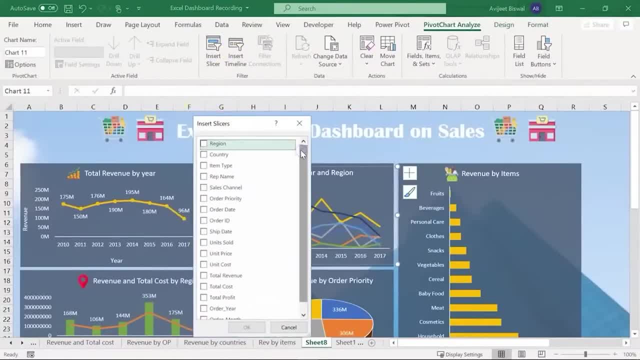 now it's giving me the list of fields present in the data set, so I'll select country, region and let's say we want to know by item type and sales channel. so these are going to be my four slicers. I'll click on that. 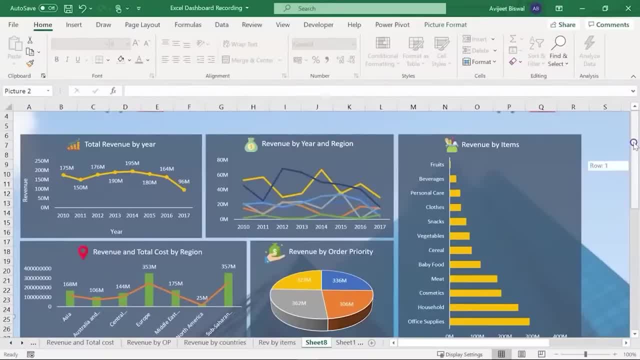 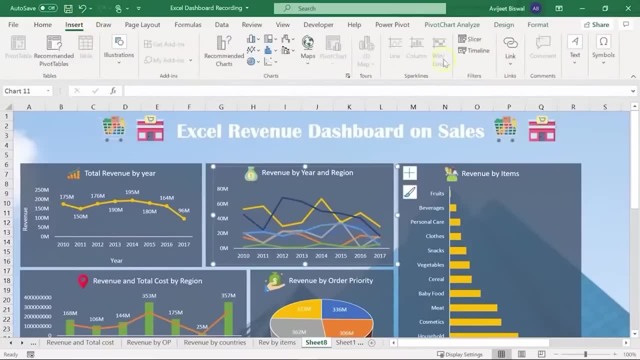 particular month. you can do that using a timeline. so i will select one of the charts and then either you can go to the insert tab- and here you can see under filters we have slicers and timeline, or if you go to the pivot chart analyze tab, here also you have 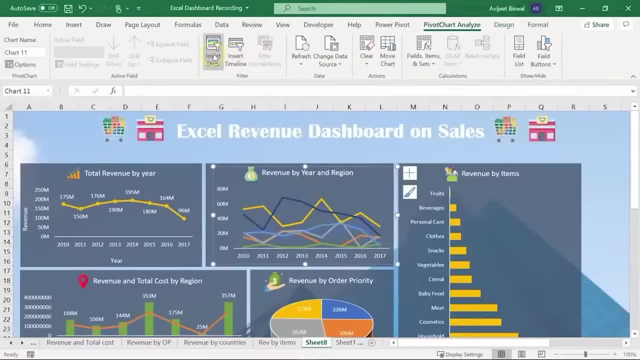 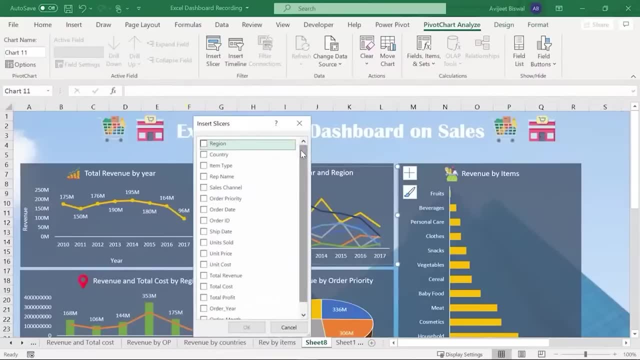 insert slicer and timeline option. so i will select insert slicer here first. now its giving me the list of fields present in the data set, so i will select country, region and lets say we want to know by item type and sales channel. so these are going to be my four. 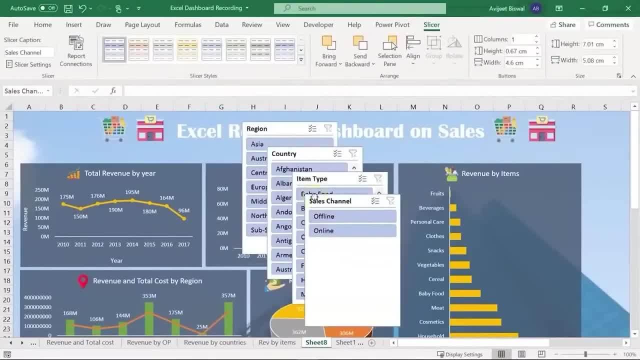 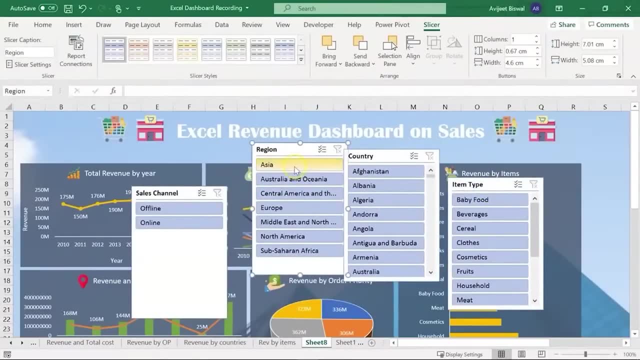 slicers. i will click on. ok, you can see it here. we have our four slicers here and these are the list of values under region. we have asia, this europe, north america and others. similarly, we have the different country names for country slicers and then for item. 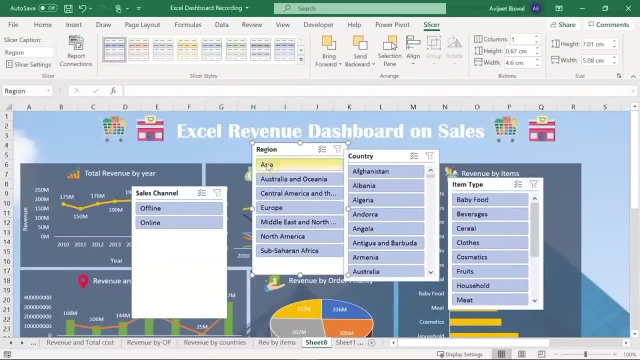 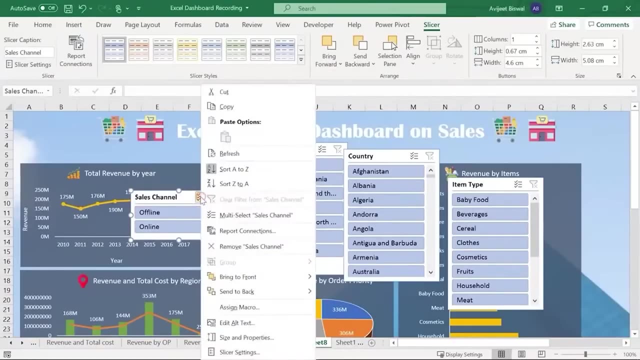 type. also, we have all the items that were present in our data set. now, moving ahead, we need to connect all the slicers to a dashboard. so what i will do is i will right click on this option and i will go to report connections. ok, so under report connections, you have. 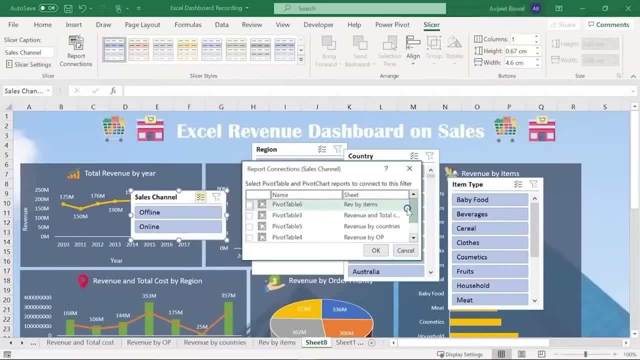 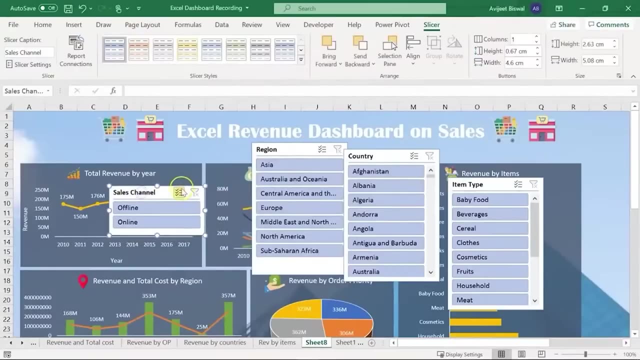 all the pivot tables that we created. currently, see, only one of the pivot table is selected, so we need to select all the pivot tables. so let me check all the pivot tables present in this workbook and click on ok, alright, now that we have connected one of our 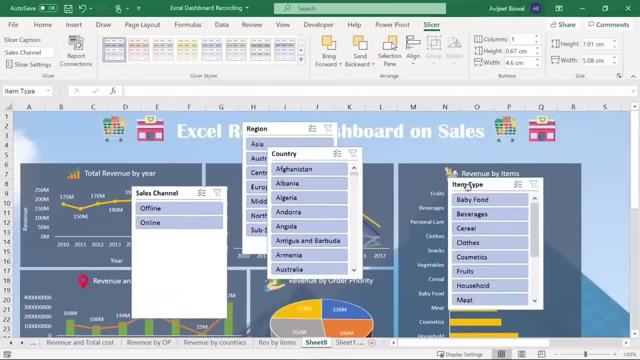 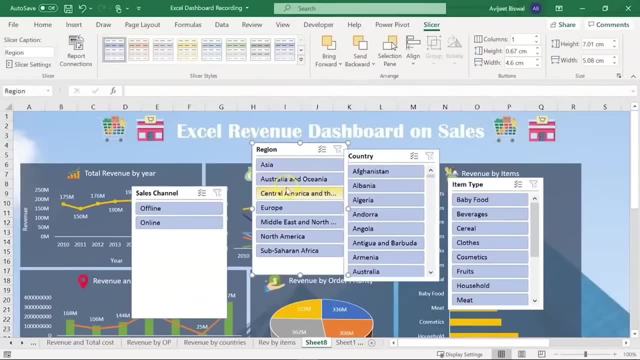 Click on OK, You can see it here. we have our four slicers here and these are the list of values. under region we have Asia, this Europe, North America and others. similarly we have the different country names for country slicers and then for item type also we have all the items that 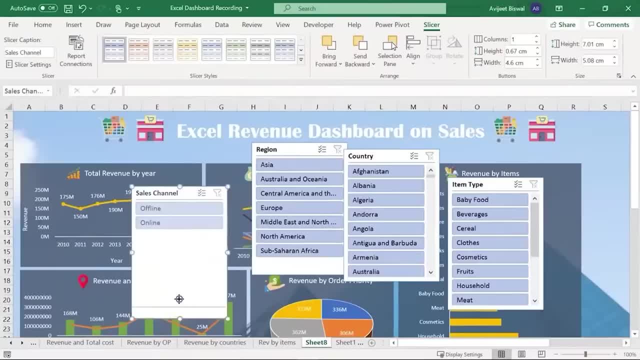 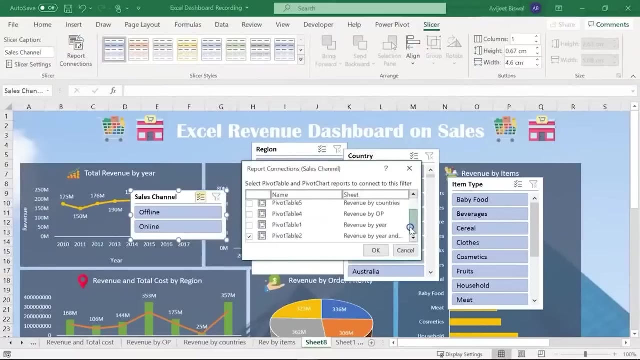 were present in our data set. Now, moving ahead, we need to connect all the slicers to a dashboard, So what I'll do is I'll right click on this option and I'll go to report connections. OK, So under report connections, you have all the pivot tables that we created. 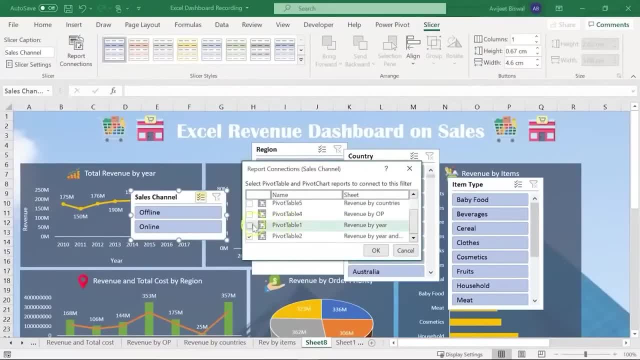 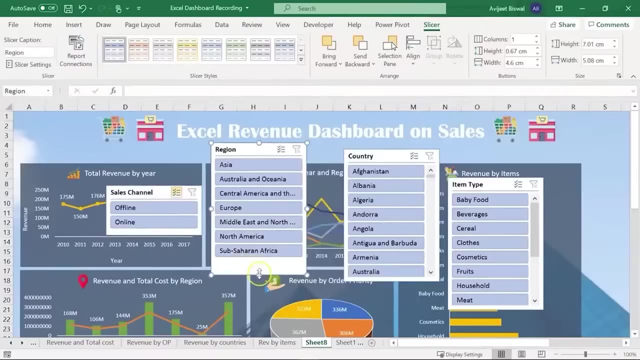 Currently see, only one of the pivot table is selected, so we need to select all the pivot tables. So let me check all the pivot tables present in this workbook and click on OK, OK, OK, All right, Now that we have connected one of our slicers, we'll now connect the other remaining slicers. 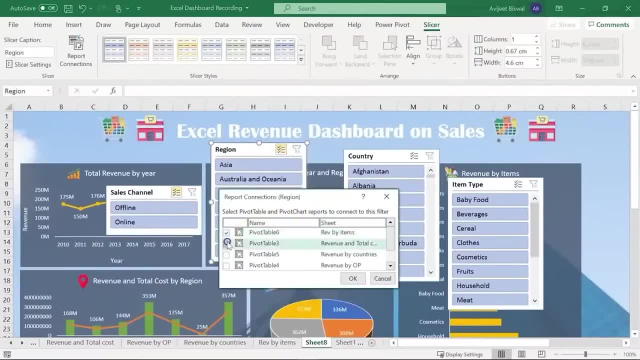 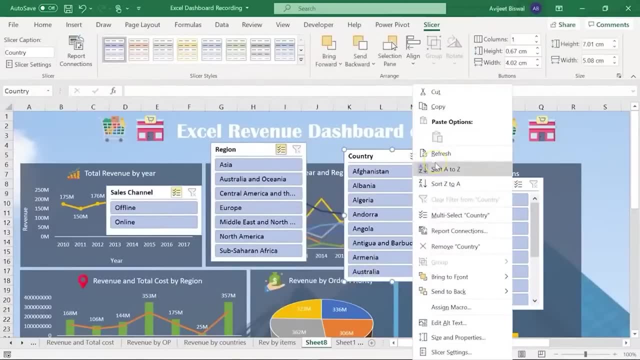 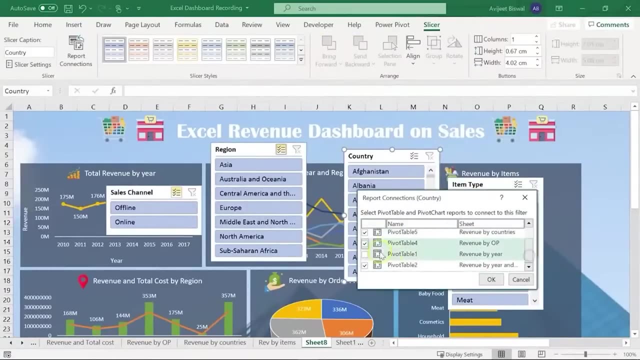 So I'll right. click on this. go to report connections and I'll check all the pivot tables present in this worksheet. Click on OK. Similarly, let's do it for the country slicer. go to report connections and let me select all the pivot tables. 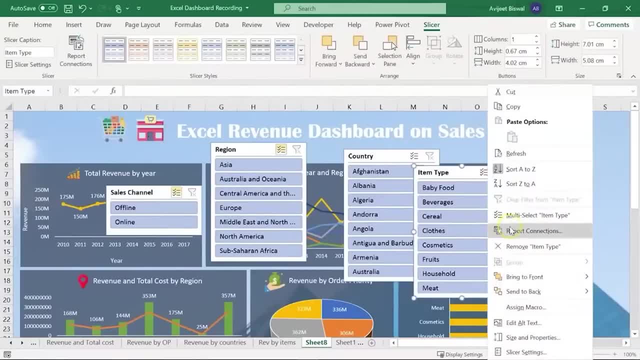 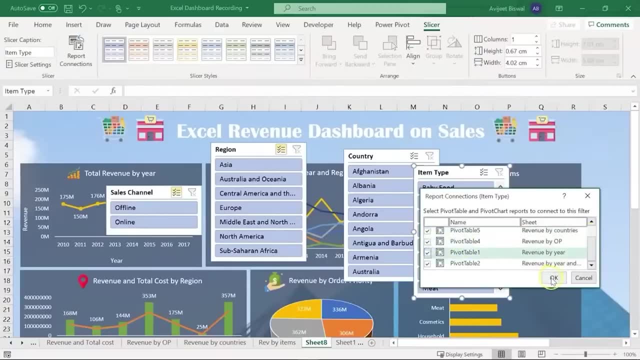 And finally We have The item type. So I'll right click, go to report connections and then I'll select all my pivot tables And let's hit OK. All right, Now let me just organize this a bit, So I'll 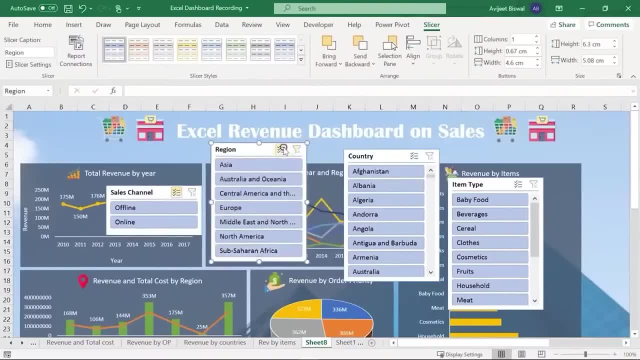 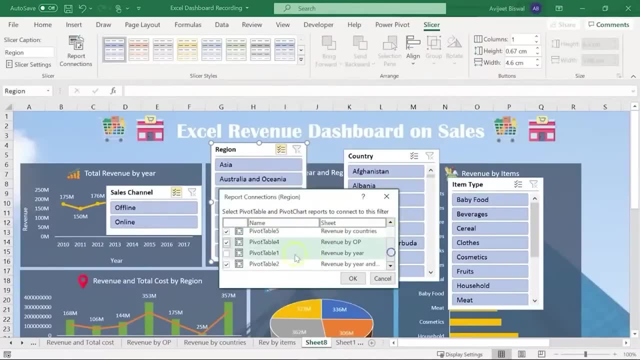 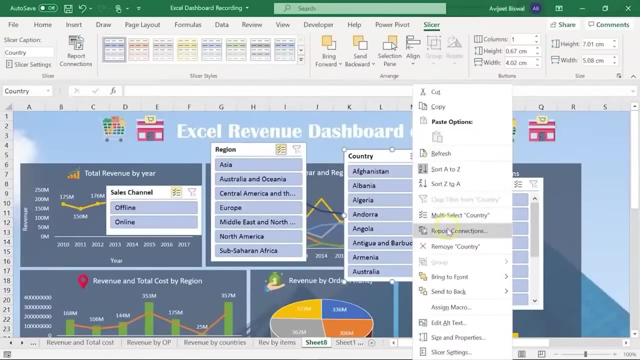 slicers. we will now connect the other remaining slicers, so i will right click on this, go to report connections and i will check all the pivot tables present in this worksheet. click on ok. similarly, let's do it for the country slicer. go to report connections and. 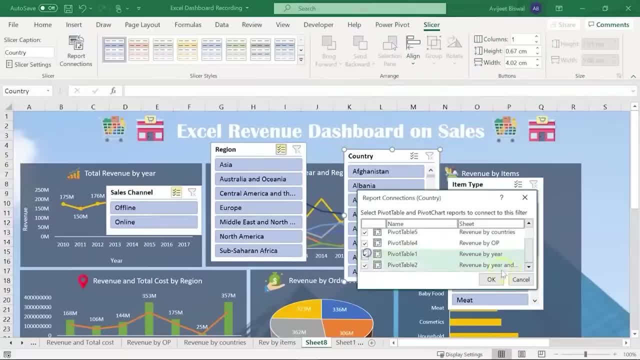 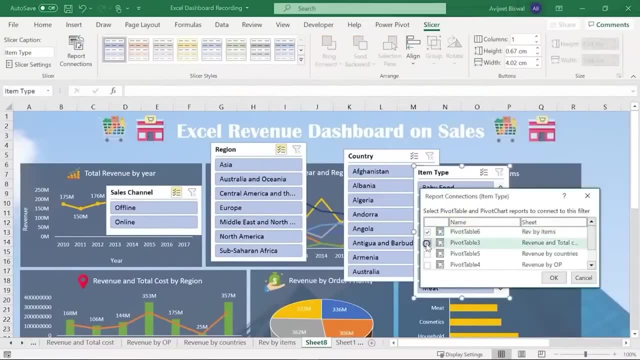 let me select all the pivot tables and finally we have the item type. so i will right click, go to report connections and then i will select all my pivot tables and let's hit ok, alright, now let me just organize this a bit. so i will place my pivot tables: 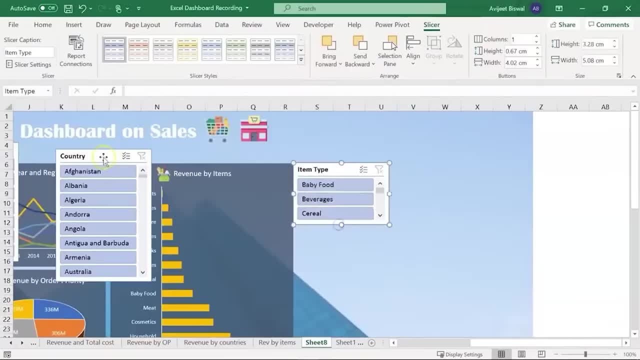 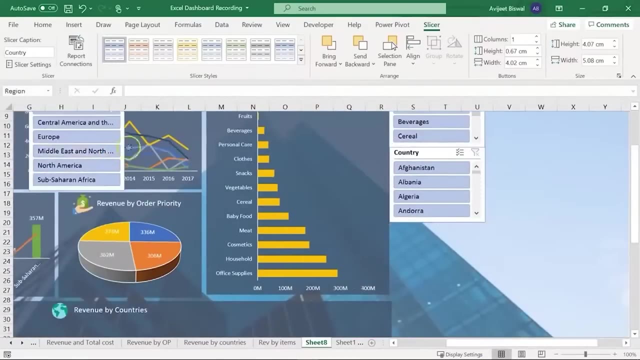 Place my pivot tables To the right. I'll just reduce the size. Let me scroll down. OK, Now I'll add My region slicer here. Similarly, I'll add my final slicer, that is, sales channel. Now, in our next dashboard, which is going to be the profit dashboard, I'll show you how to. 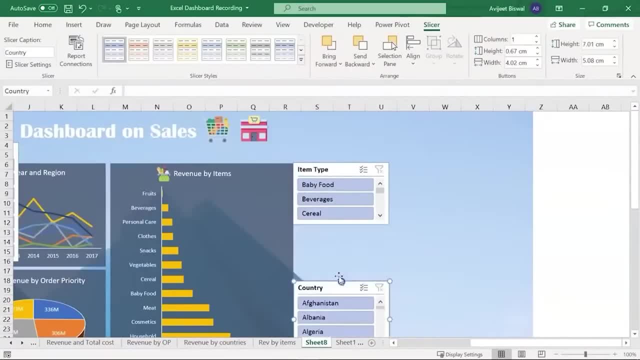 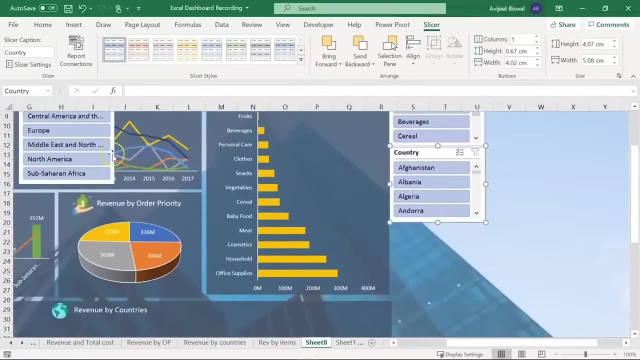 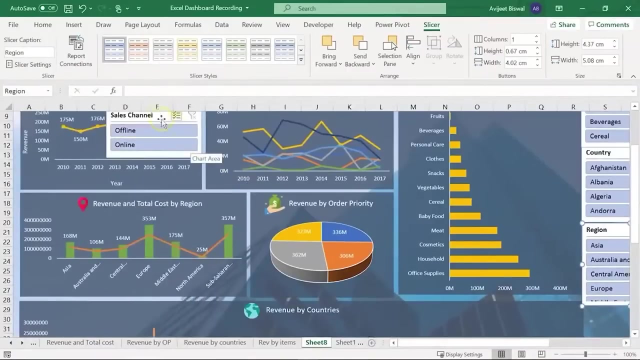 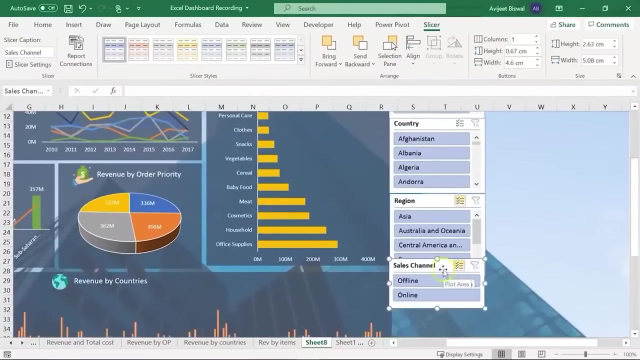 to the right. i will just reduce the size. let me scroll down. i will add my region slicer here. similarly, i will add my final slicer, that is, sales channel. now, in our next dashboard, which is going to be the profit dashboard, i will show you how to add a timeline. 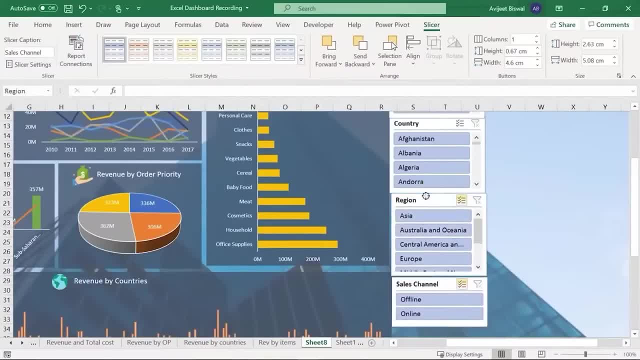 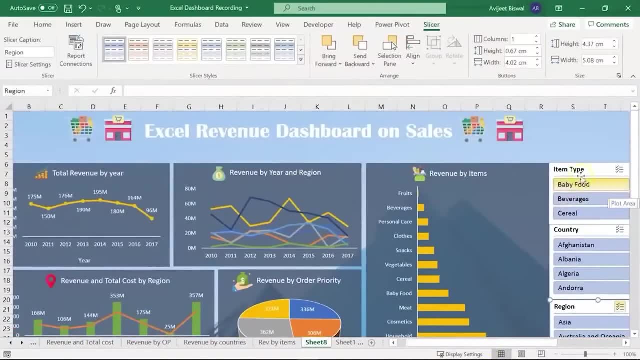 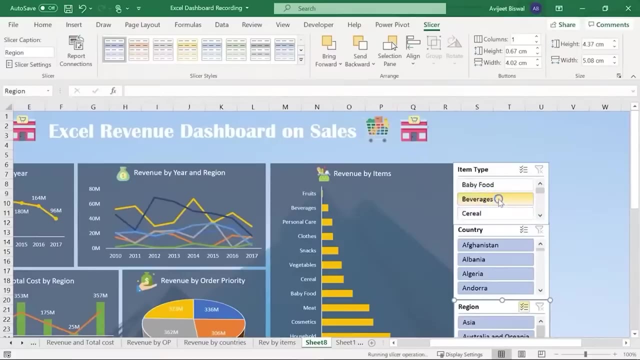 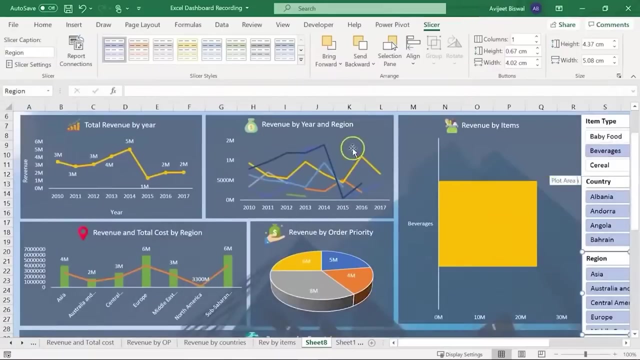 alright, now i have arranged all my slicers. so let's say you want to find the revenue that was generated for an item type, let's say beverages, so you can just select beverages here and all your charts show the respective revenues. so you have the total revenue. 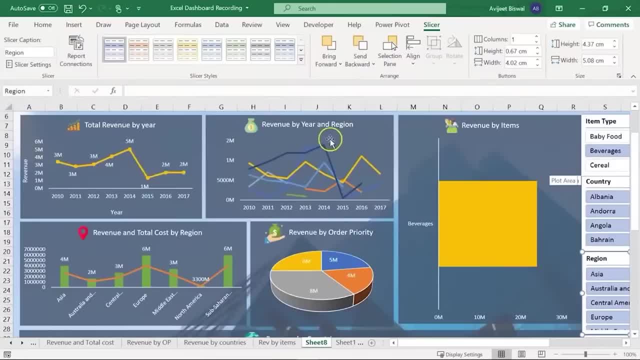 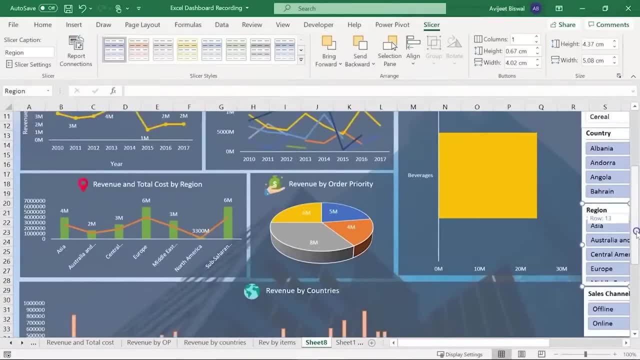 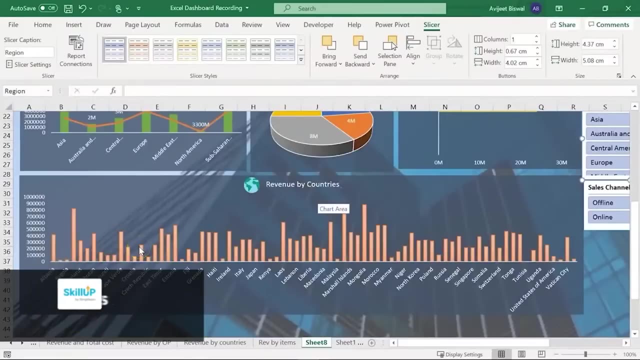 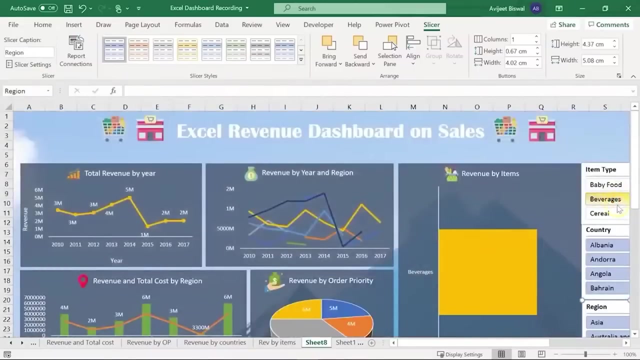 by year for beverages only. similarly, here you can see the revenue by year and region only for beverages, item type. if i scroll down now, this chart represents the revenue that was generated in each of the countries only for item type: beverages. let me just uncheck it, alright. 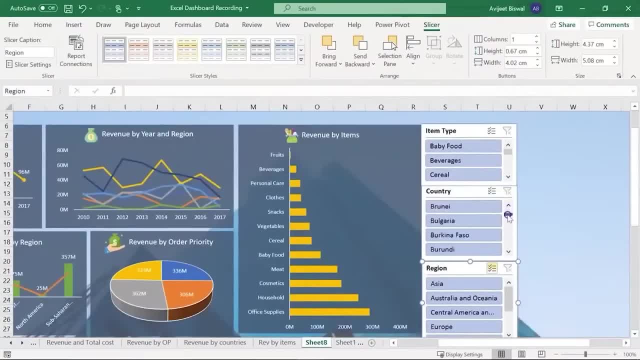 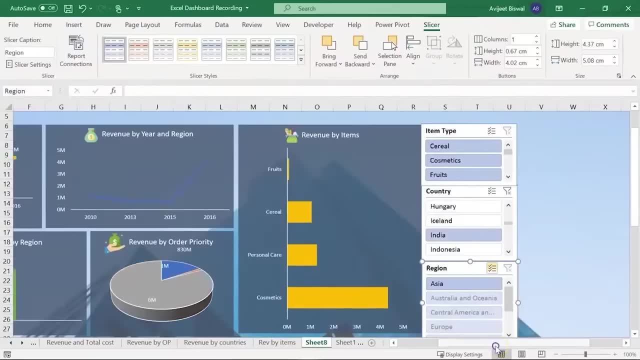 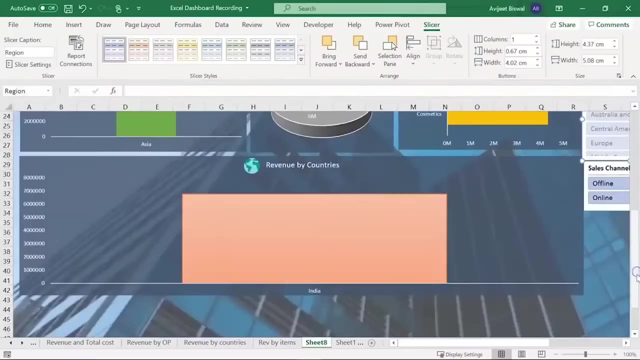 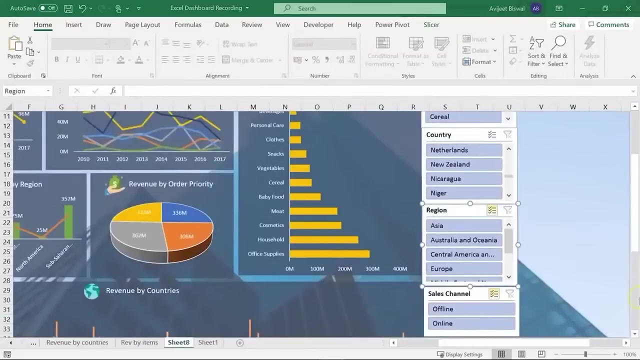 let's say you want to see the revenue generated for a country like India, so i have selected India here and now you can see my graph has changed. only for country India. you can see here it is showing only for India now. now. similarly, you can also filter your revenues based on the different. 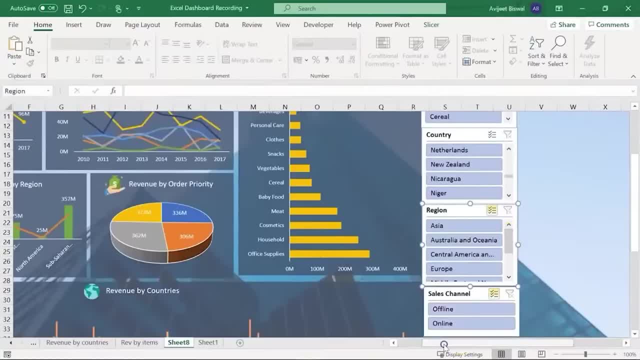 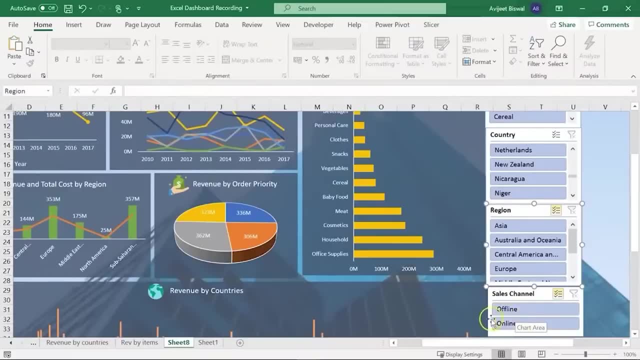 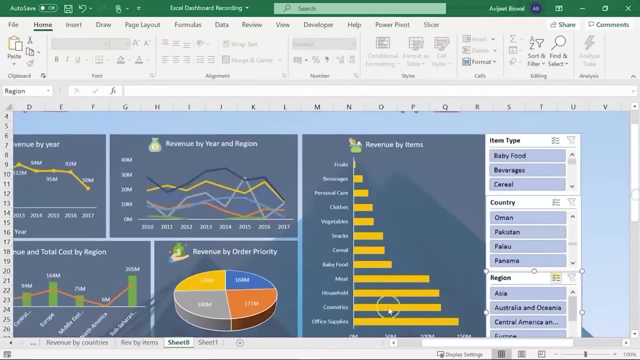 regions. let's say you want to know the revenue generated based on sales channel. so we have two sales channel, that is, offline and online. suppose you want to know the revenue generated offline, so i will just select offline. you can see the values have changed. so these were the revenues. 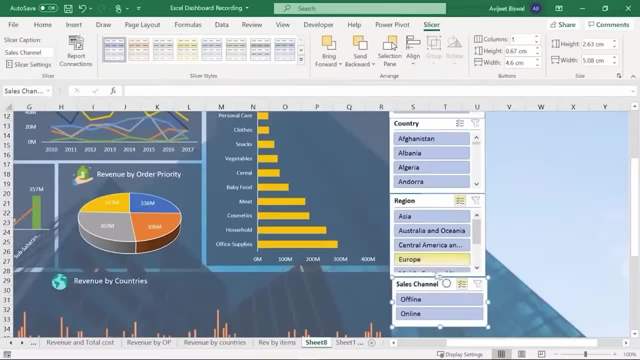 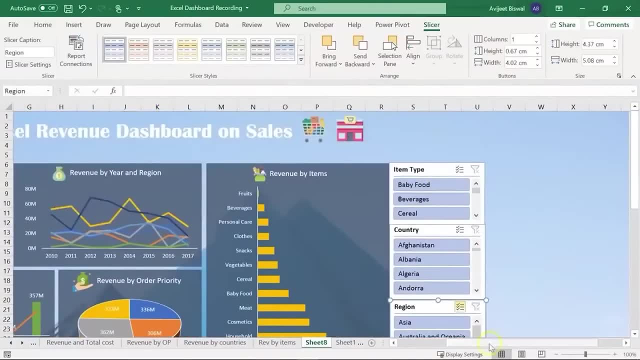 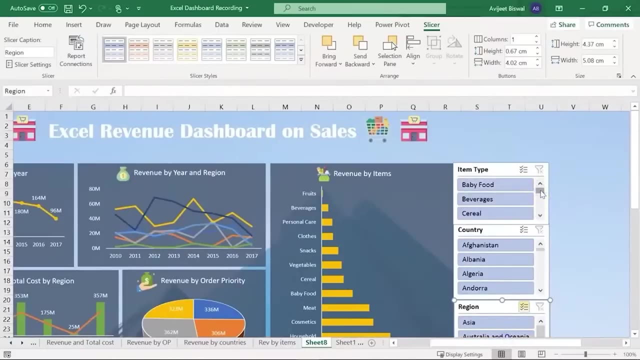 add a timeline. All right, Now I have arranged all my slicers, OK? So let's say you want to find the revenue that was generated for an item type, Let's say beverages, So you can just select beverages here And 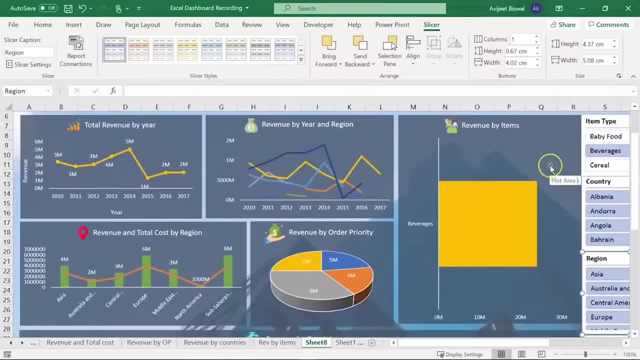 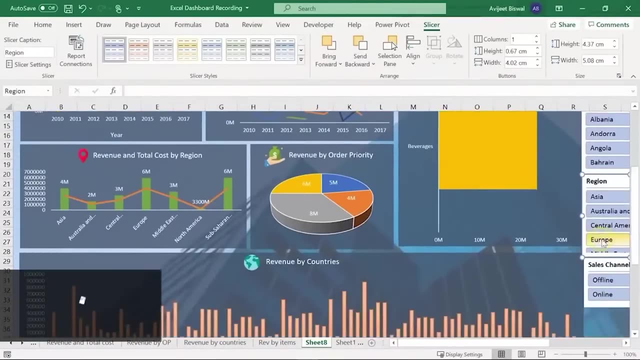 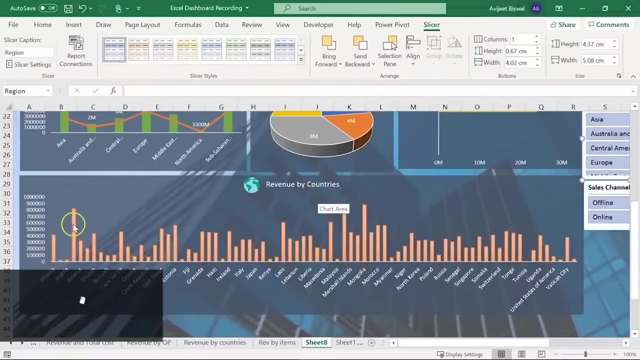 All your charts, So the respective revenues. So you have the total revenue by year for beverages only. Similarly, here you can see the revenue by year and region only for beverages. item type: If I scroll down Now, this chart represents the Revenue that was generated in each of the countries only for item type: beverages. 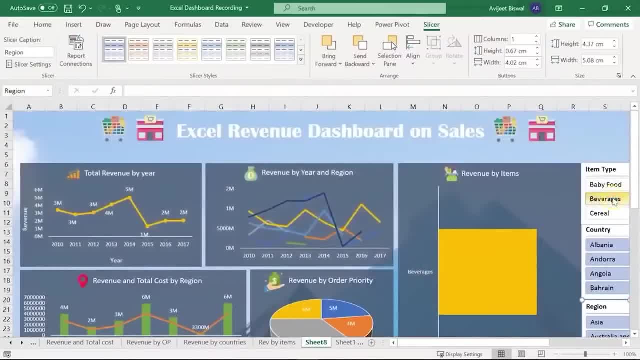 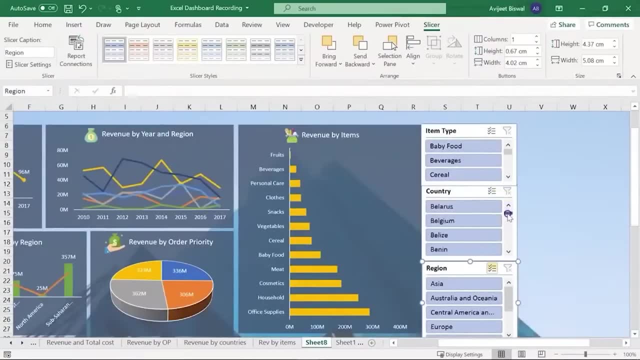 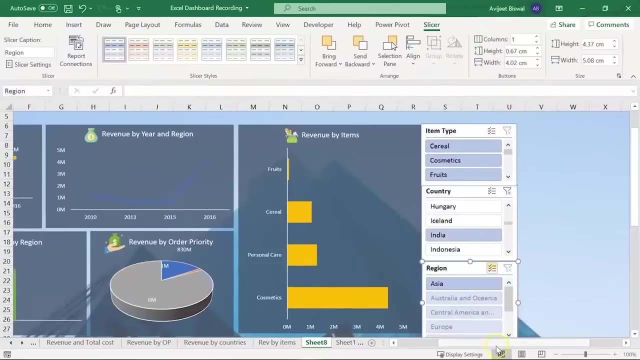 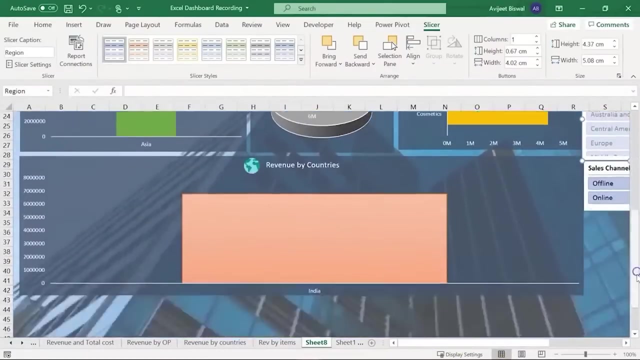 Let me just uncheck it. All right, Let's say you want to see The revenue generated for a country like India, So I have selected India here And now you can see My graph has changed. only for Country India, You can see here it is showing only for. 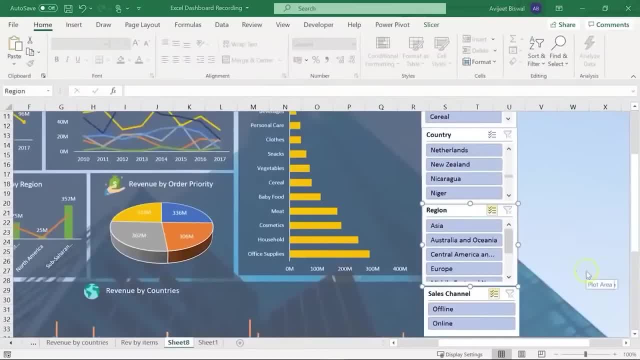 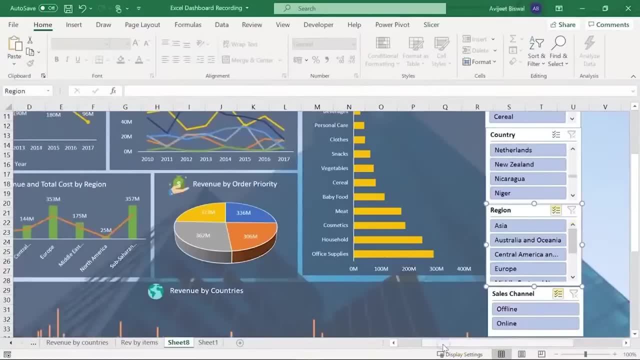 India now. Now, similarly, you can also filter your revenues based on the different regions. Let's say you want to Know the revenue generated Based on sales channel. So we have two sales channel, that is, offline and online. Suppose you want to know the revenue generated offline. 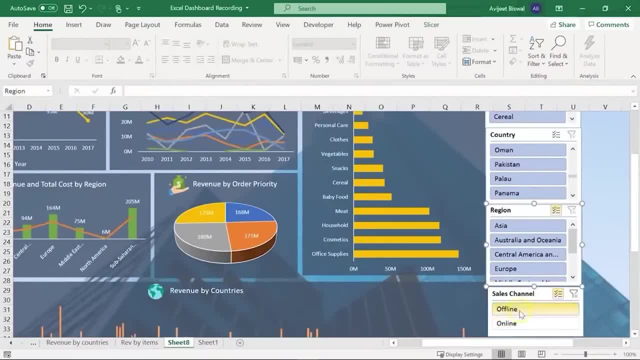 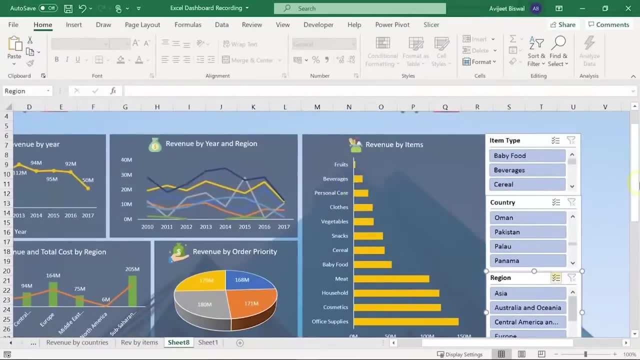 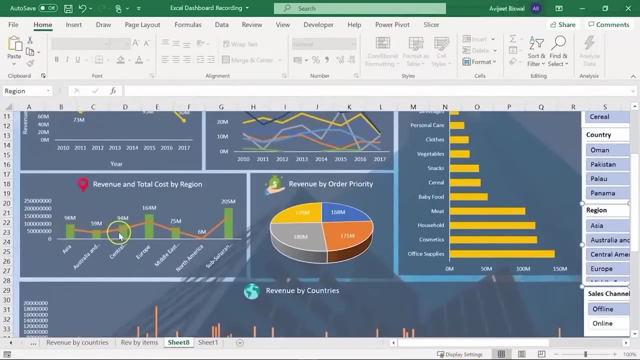 So I'll just Select Offline. you can see The values have changed. So these were the revenues generated for each of the items, only for offline. If you See here Now, these were all the Offline sales for the different regions. 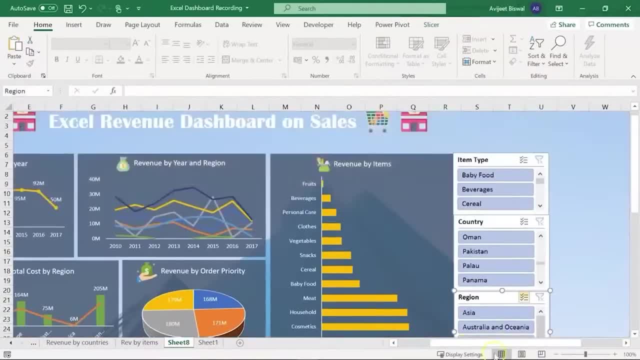 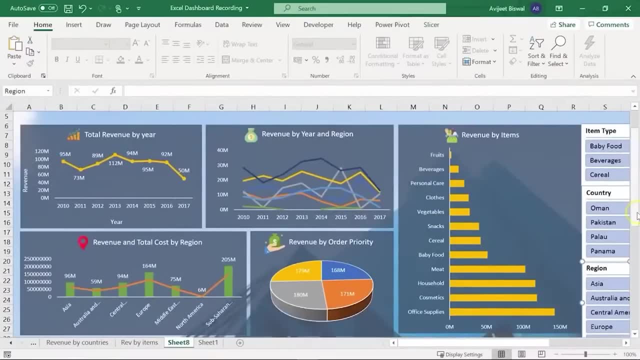 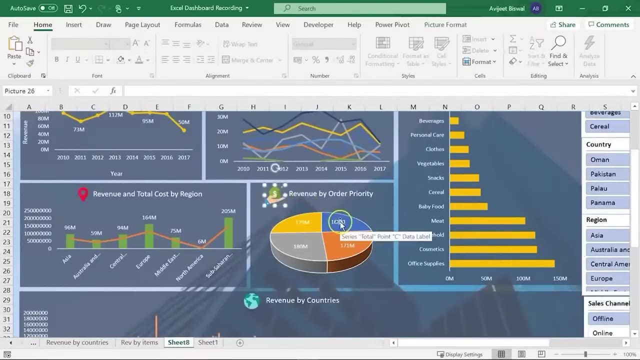 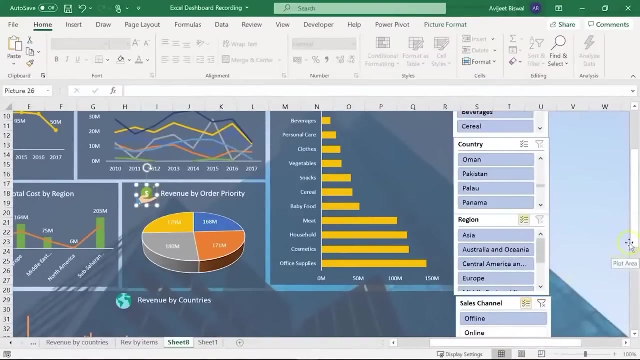 So This is Our entire Excel revenue dashboard on sales. We created multiple charts and graphs, Then we applied Different formatting, we added Different icons, Then we formatted the labels also. Next we added Slicers And Finally we saw how we could. 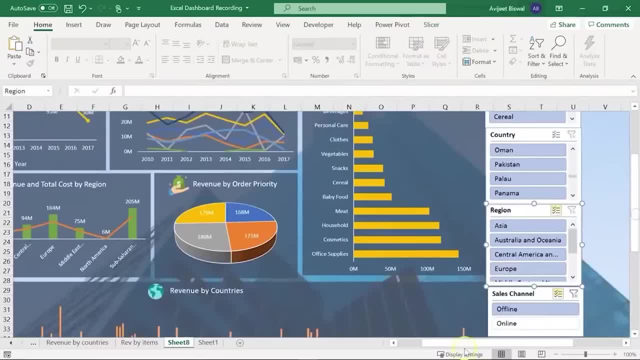 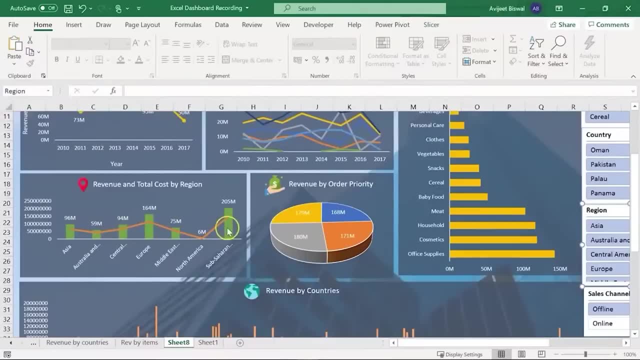 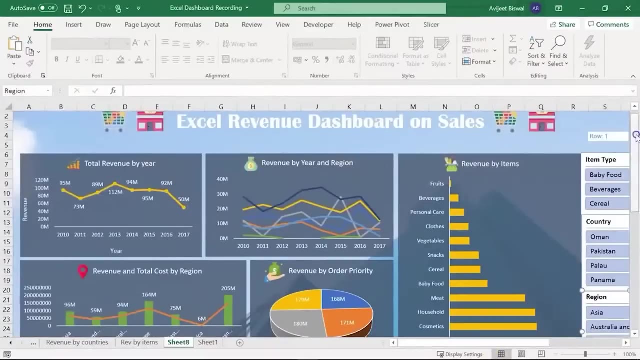 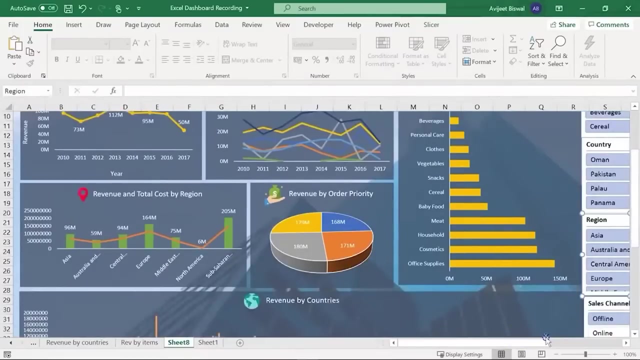 generated for each of the items only for offline. if you see here now, these were all the offline sales for the different regions. so this is our entire excel revenue dashboard on sales. we created multiple charts and graphs, then we applied different formatting. we added different icons, then we formatted. 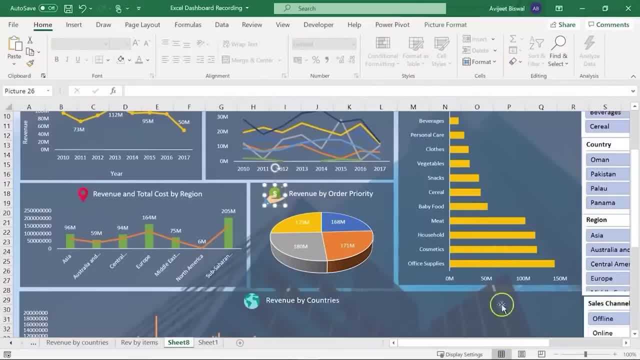 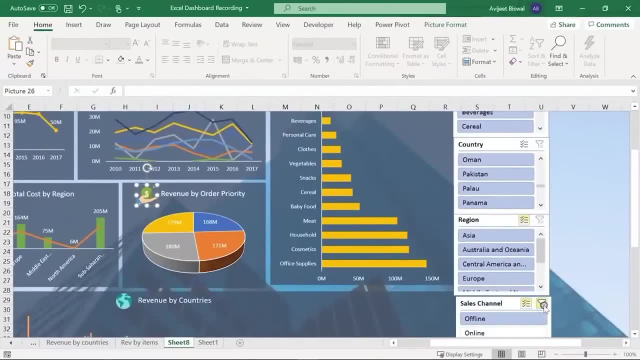 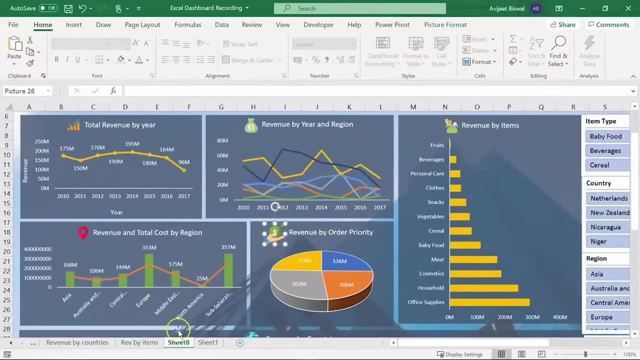 the labels also. next, we added slicers and finally, we saw how we could filter our data based on these slicers. likewise, now we are going to create a profit dashboard based on the same data. so before moving ahead, let me rename this sheet as revenue dashboard. i will write: rev. 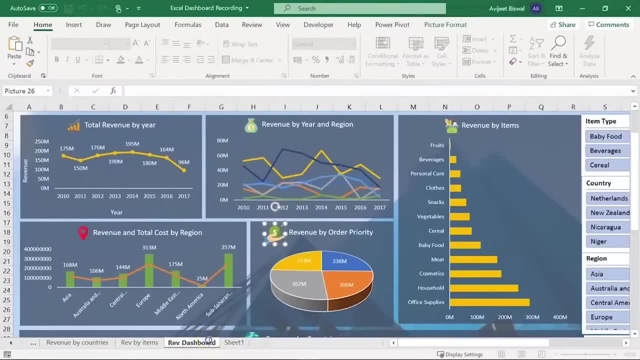 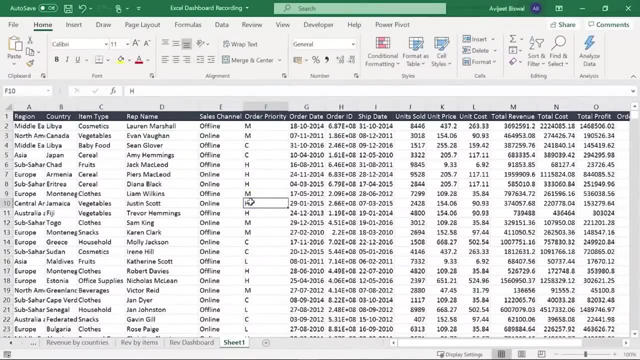 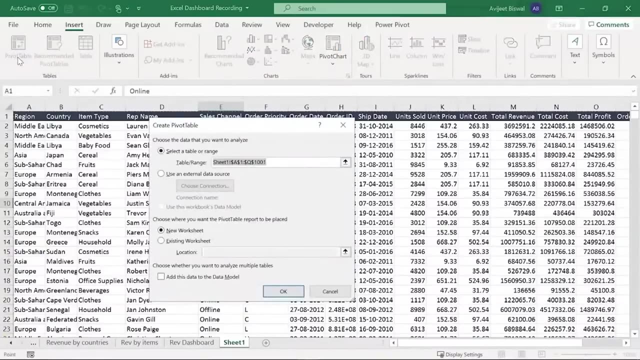 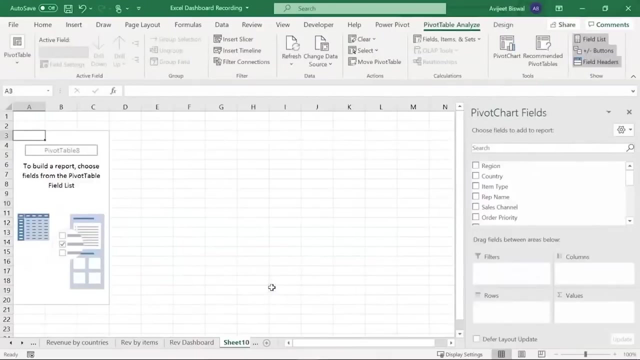 dashboard. ok, now we will move to our data sheet and start creating our pivot tables and pivot charts for the profit dashboard also. right, so let me go ahead and create my first pivot table. so i will create a new worksheet. this time i am going to create a line chart. 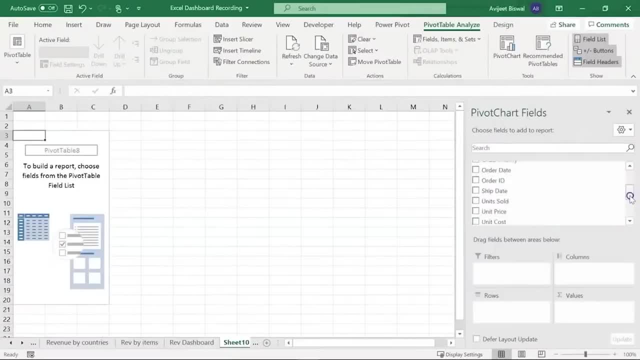 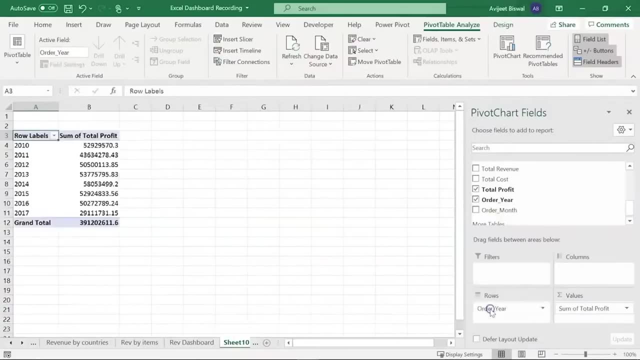 to visualize the profit for each year. so i will drag my total profit column to values and my order year to rows. so here you can see. we have our pivot table ready. now you can sort this data to get an idea as to which year had the highest profit. 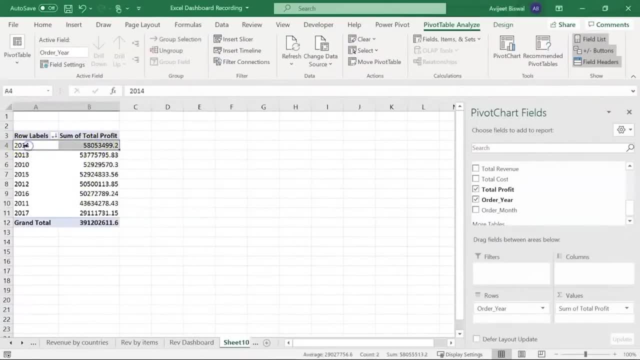 and which year had the lowest profit. so from this pivot table you can see, since i have sorted this data in descending order- so 2014 had the maximum amount of profit and 2017 had the least amount of profit. i will just do control z to undo it. alright. 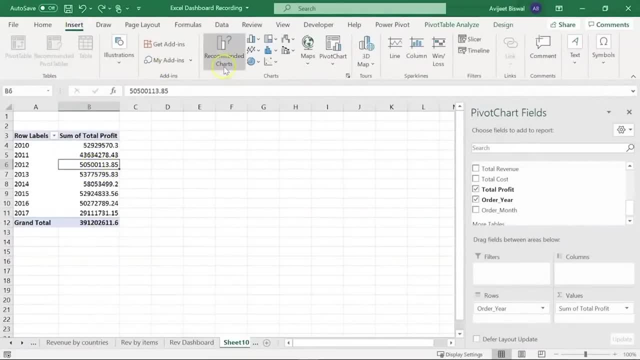 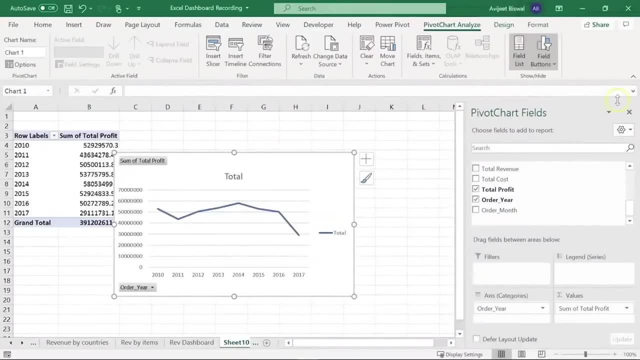 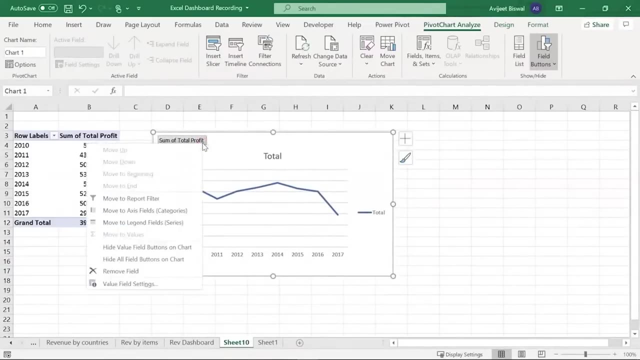 now, based on this pivot table, let me go ahead and create my pivot chart. so i will go to recommended charts and click on a line chart. so this is the preview of the chart i will click on. ok, let me close this. similarly, we are going to edit this chart. 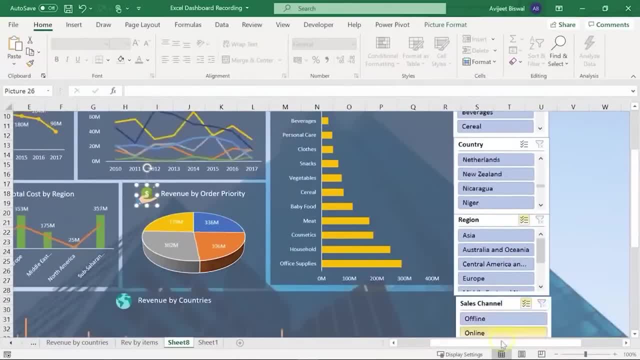 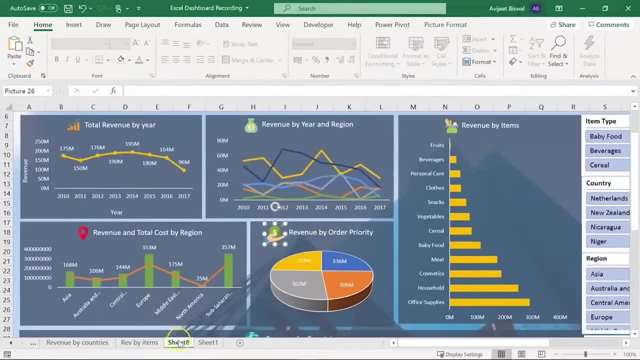 Filter our data based on these slicers. Likewise, Now we are going to create a profit dashboard Based on the same data. So before moving ahead, Let me Rename this Sheet as Revenue dashboard. I'll write: REV Dashboard. 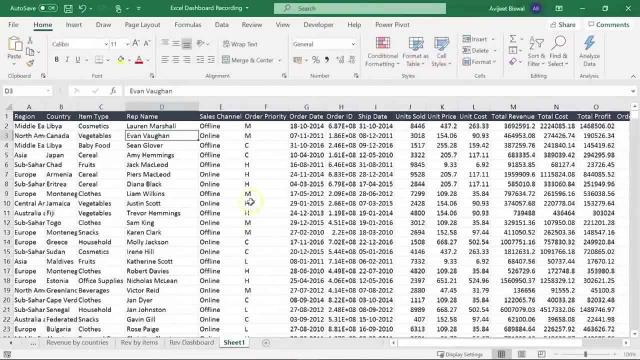 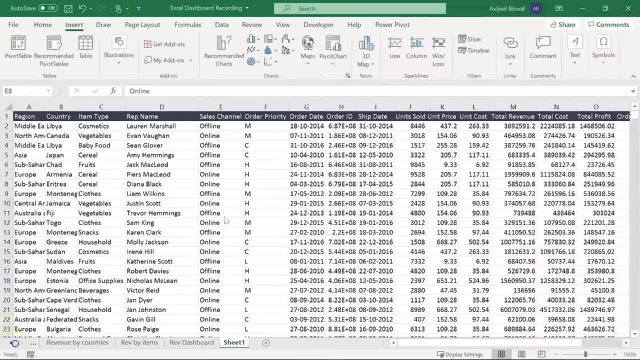 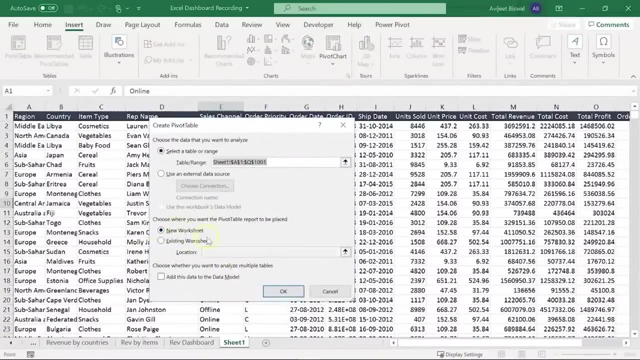 Okay, Now We move to our data sheet And Start creating a pivot tables and pivot charts for the profit dashboard. All right, So let me go ahead and create my first pivot table. So I'll create A new worksheet. 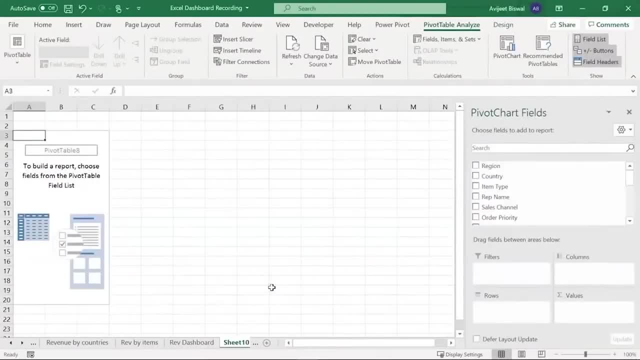 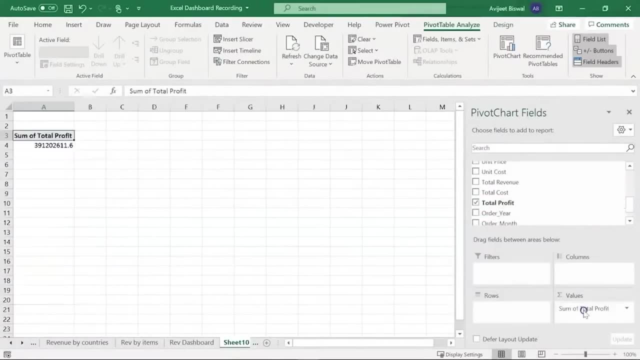 This time I'm going to create a line chart To visualize the profit for each year. So I'll drag my Total profit column To values And My order year To rows. So here you can see, we have our. 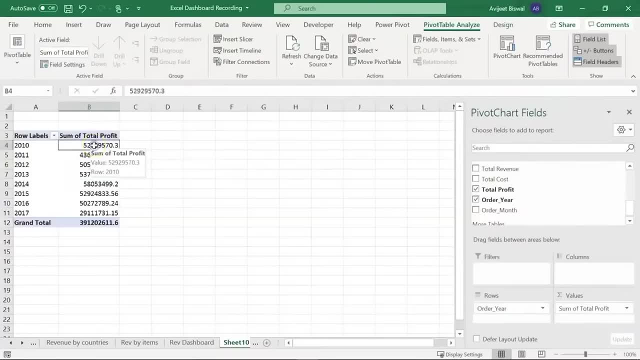 Pivot table ready Now. you can sort this data To Get an idea As to which Year had the highest profit And which year had the lowest profit. So from this pivot table You can see, Since I've sorted this data in. 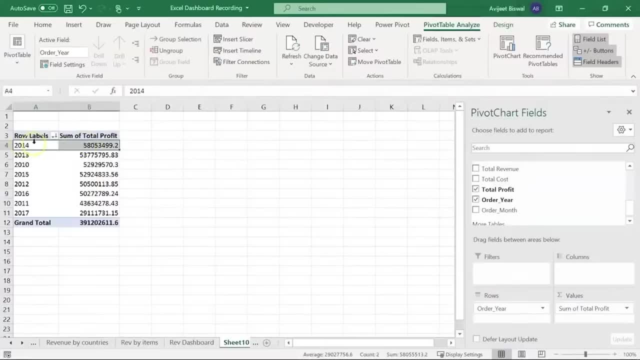 Descending order. So 2014.. Had the maximum amount of profit And 2017.. Had the least amount of profit. I'll just Do control Z to undo it All right. Now, based on this pivot table, Let me go ahead and create my pivot chart. 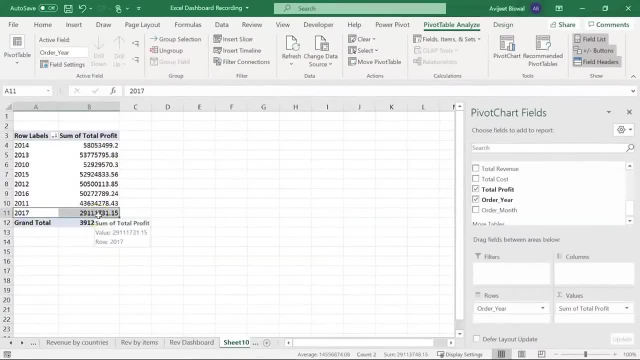 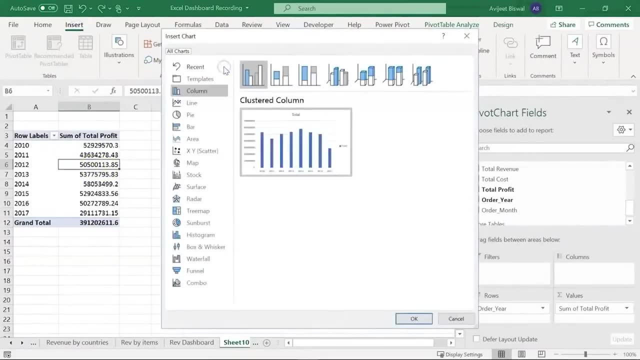 So I'll go to recommended charts And click on a line chart. So this is the preview of the chart And I'm going to Create My Pivot chart. So I'll go to recommended charts And Click on a line chart. 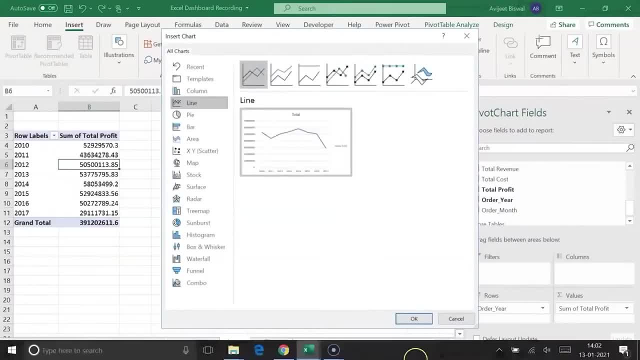 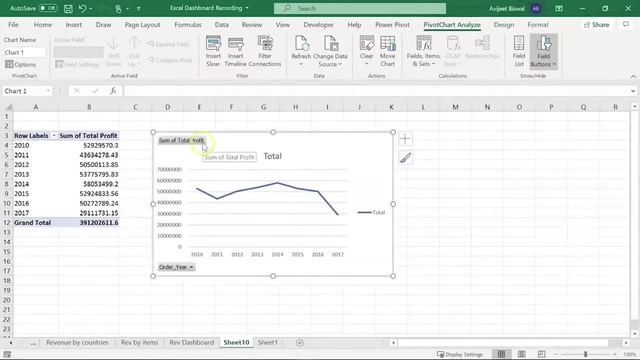 So this is the preview of the chart And I'm going to Create My Pivot chart. So this is the preview of the chart I'll click on. Okay, Let me close this. Similarly, We are going to: 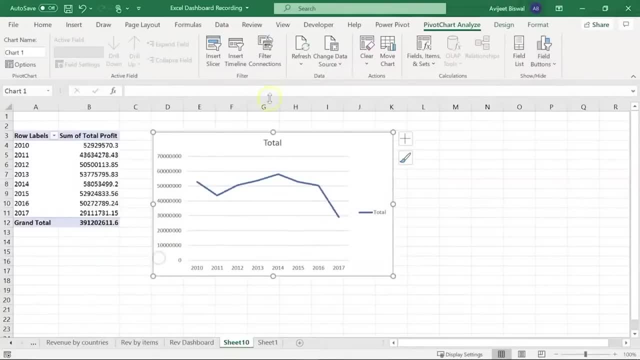 Edit this Chart Now. So first I'll hide all the field buttons present on the chart And I'll Rename the chart Title as Total Profit By Year. Next I'm going to Remove the 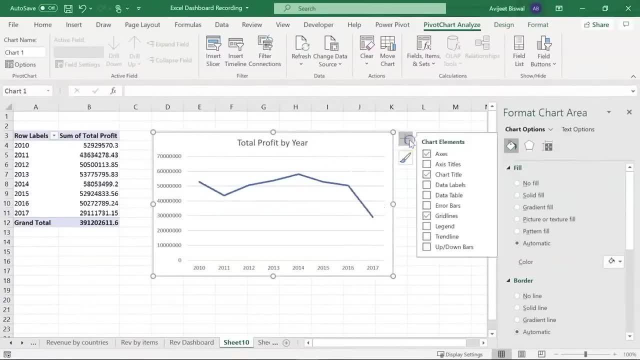 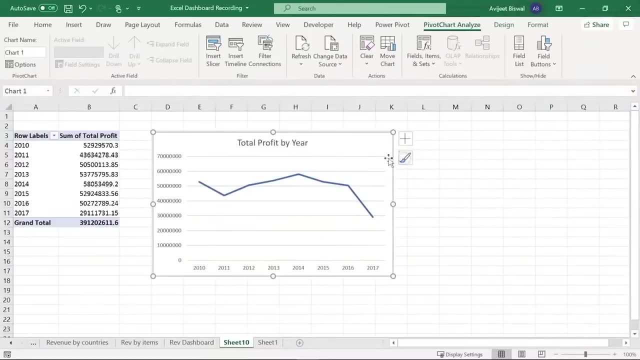 Legend, So I'll delete this. Let's do Some more Formatting, So I'll go to style, And This time I'm going to select My Style Type. Okay, And If you want, You can. 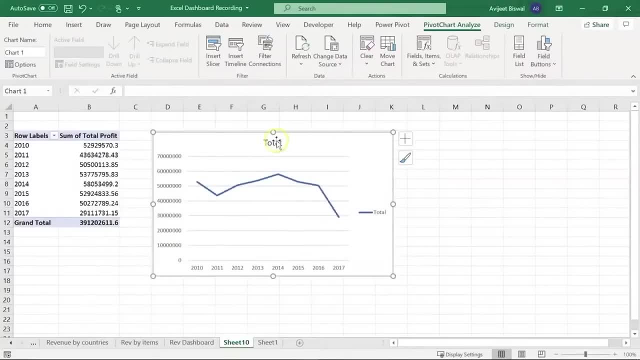 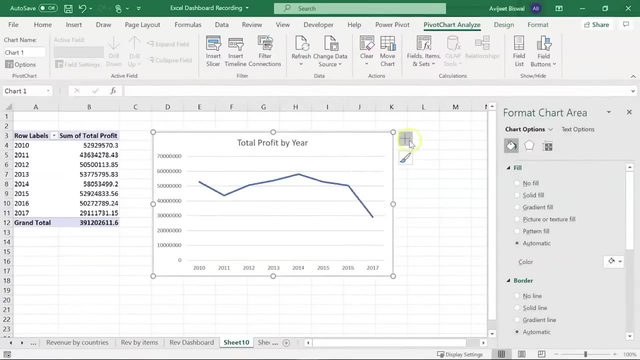 now. so first i will hide all the field buttons present on the chart and i will rename the chart title as total profit by year. next i am going to remove the legend, so i will delete this. let's do some more formatting, so i will go to style. 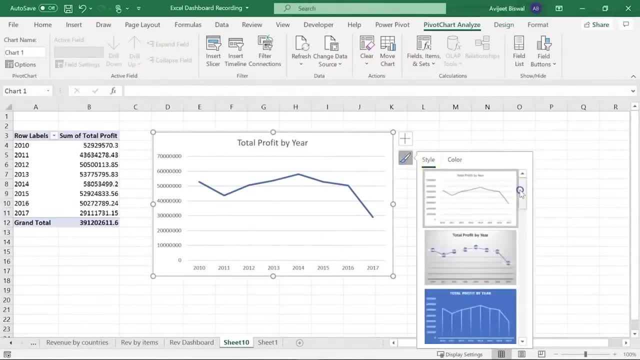 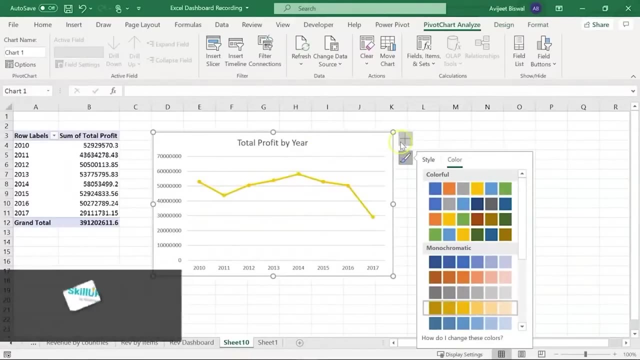 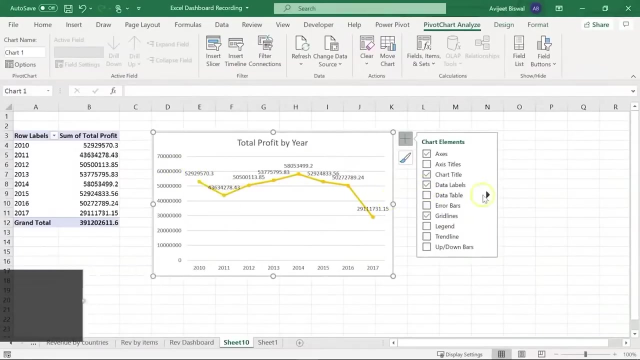 and this time i am going to select my style type. ok, and if you want, you can choose the colors as well. for the time being, let's have this yellow color. next, let me add the data labels. so again, if you see, here this is not formatted properly, so let's go ahead. 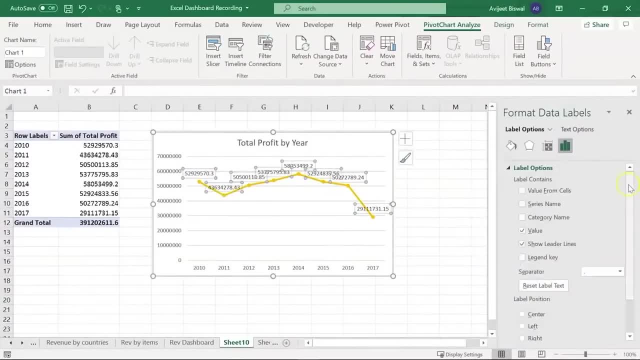 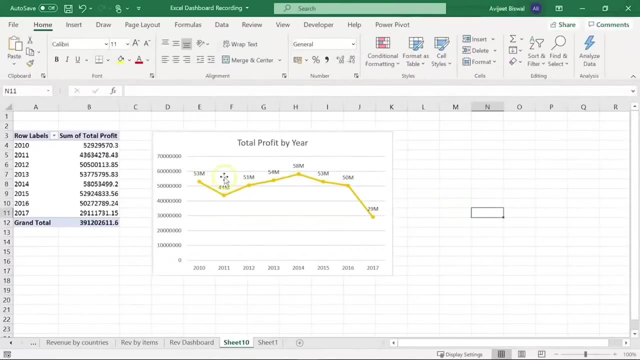 and format the data labels. so i will click on number and i will select custom here and the type i am going to select is in millions and i will click on close. so here you can see, we have our line chart ready, which shows total profit by year. 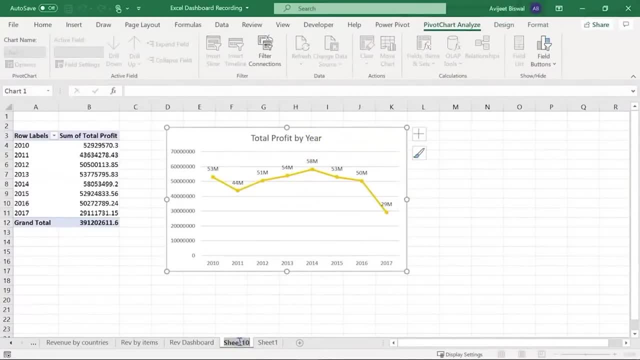 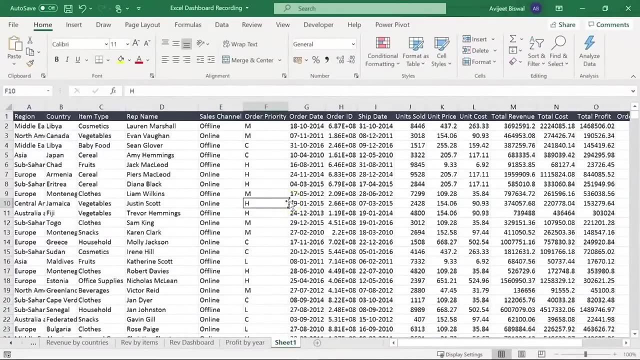 let's rename this sheet as profit by year. alright, now let's move back to our data sheet again. next we are going to show the total profit by countries. for this i am going to create a map, so let me first create my pivot table. so i will go to insert and i will 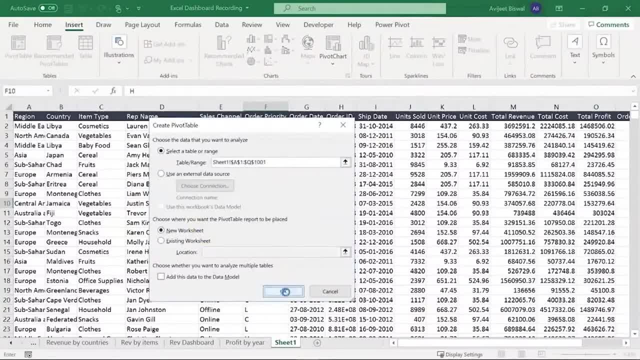 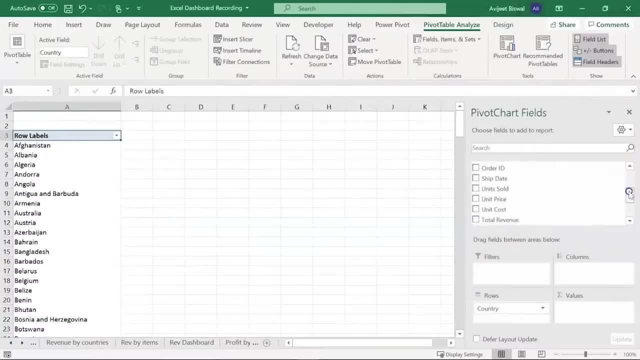 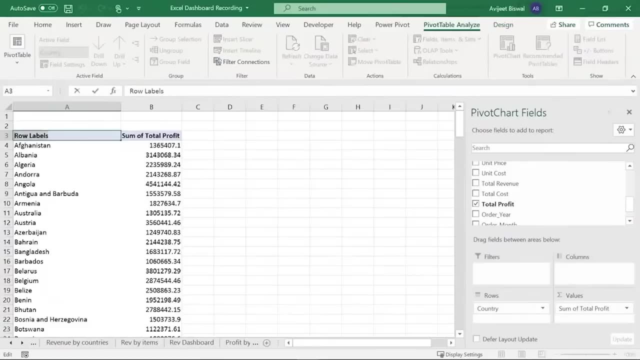 click on pivot table. let me click on ok, since i want the country name. so i will select country under rows and then i have my total profit under values. the next thing i am going to do is i will just rename the row labels as countries and then 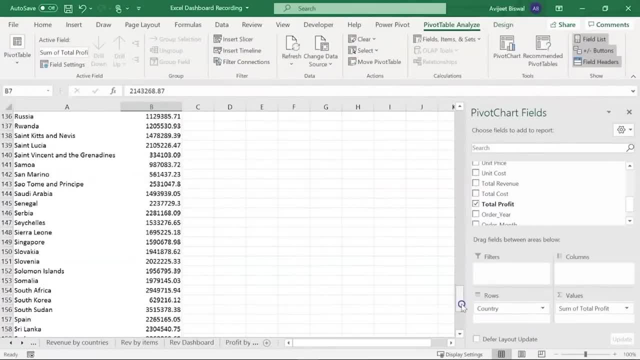 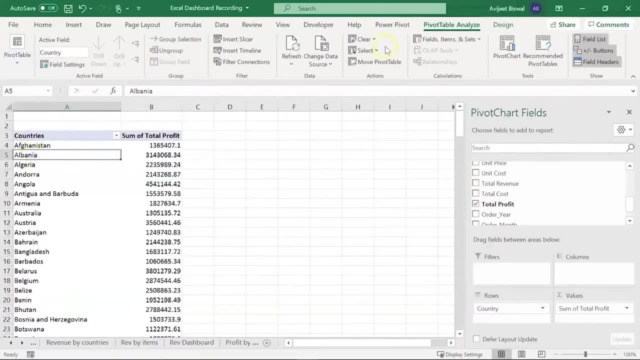 i am going to delete the grand total, which you can see at the bottom. so here we have the grand total. let me just delete the grand total. so i am going to select this pivot table. go to the design tab. here we have subtotals and grand totals. 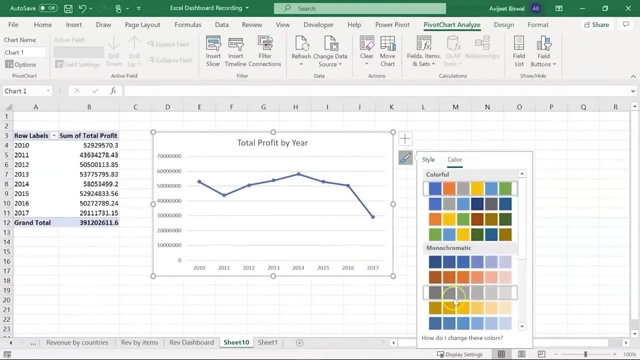 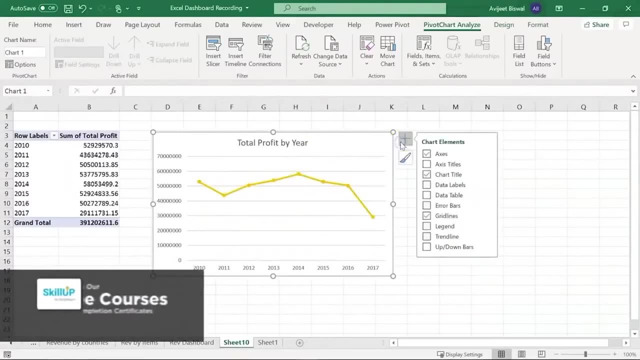 Choose the colors as well. For the time being, Let's have This Yellow color. Next, Let me add the Data labels. So again, If you see, here This is not Formatted properly, So let's Go ahead. 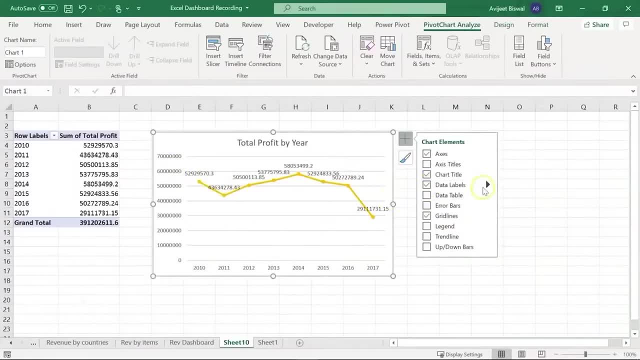 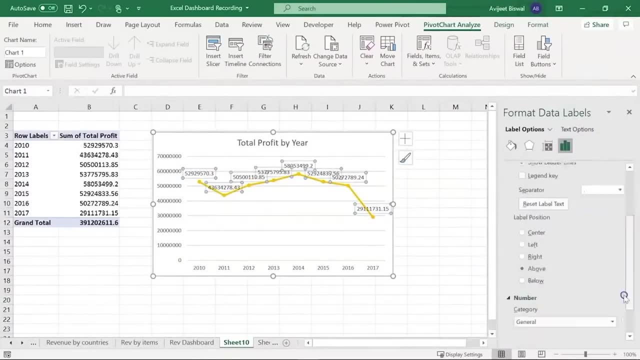 And Go ahead And Format The Data Labels. So I'll Click on Number And I'll Select Custom Here And The Type I'm Going To Select. 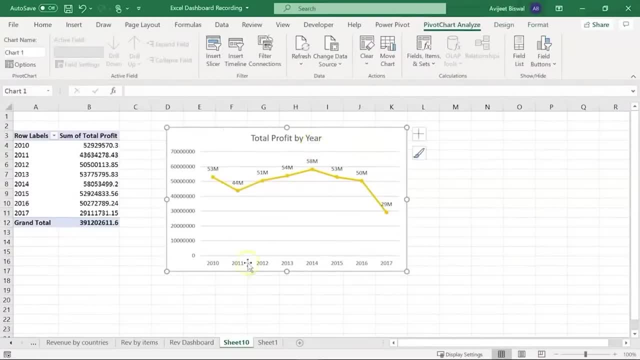 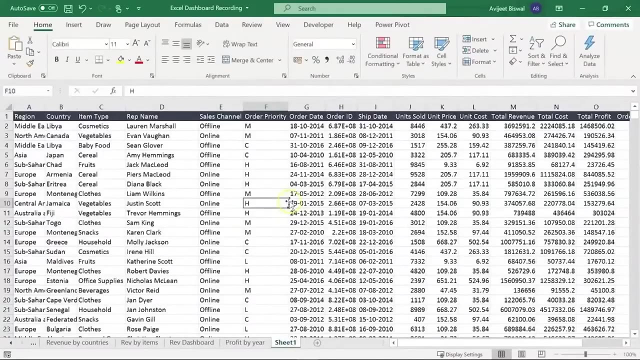 Is In Millions And I'll Click On Close. So Now Let's Go To The Data Labels. So Let's Go Back To Our Data Sheet. 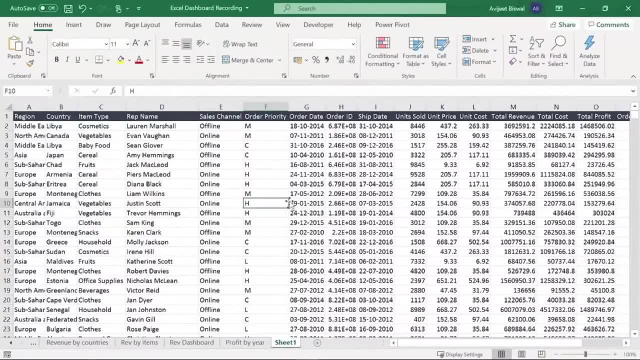 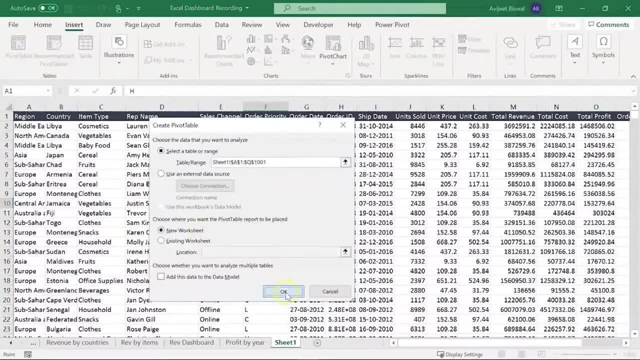 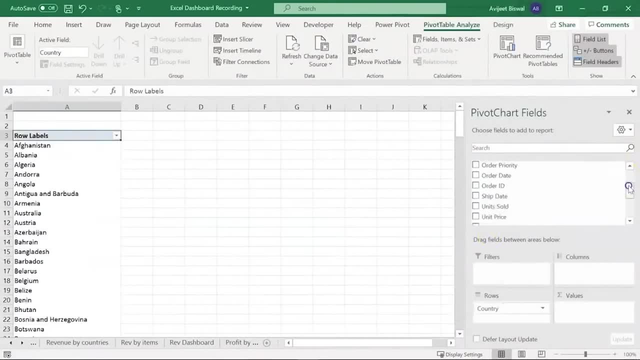 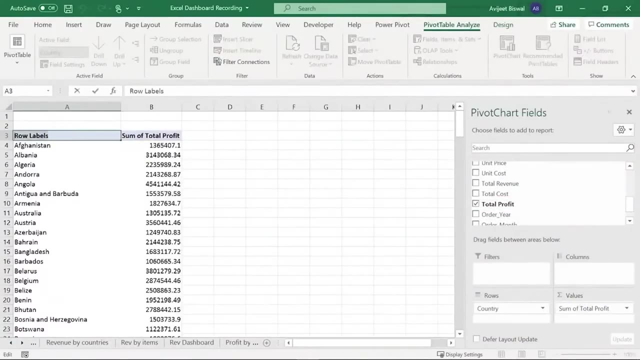 Again. Next We're Going To Show The Total Profit By Countries. For This I'm Going To Select Country Under Rows And Then I Have My. 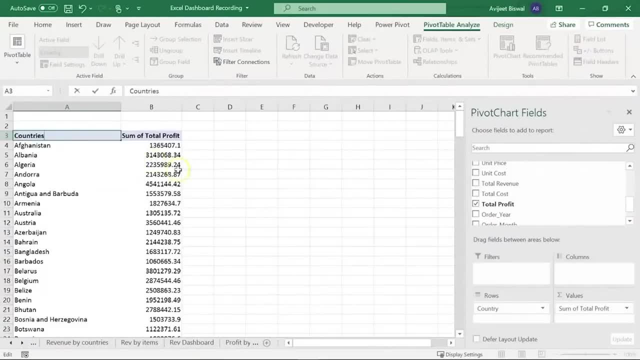 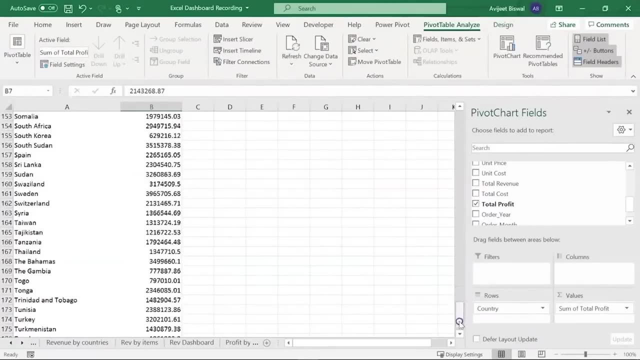 Total Profit Under Values. The Next Thing I'm Going To Do Is I'll Just Rename The Row Labels, As Here We Have Subtotals And 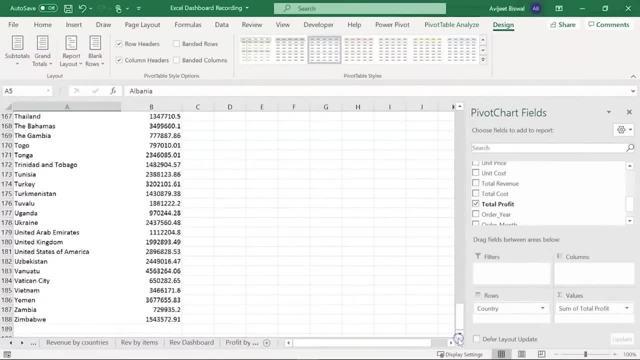 Grand Totals. I'll Switch Off The Grand Total. Let Me Just Verify It Again. I'll Scroll Down. You See, The Grand Total Has Gone. 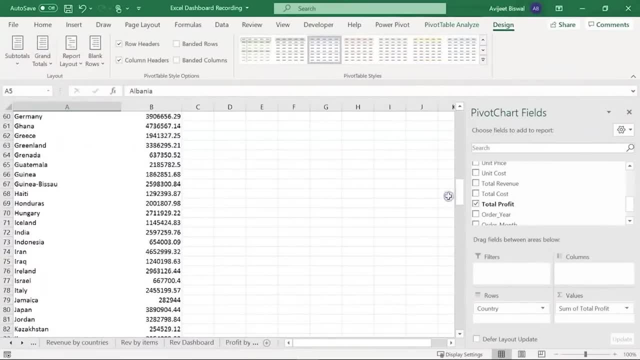 i will switch off the grand total. let me just verify it again. i will scroll down. you see the grand total has gone now. alright, now we want to create a map out of this. the way to do is: i am going to select my data, copy it. i will go on top. 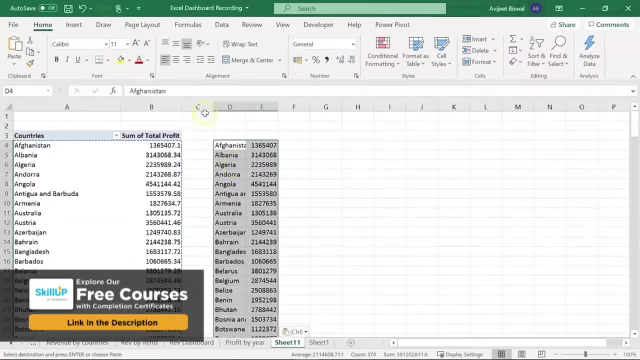 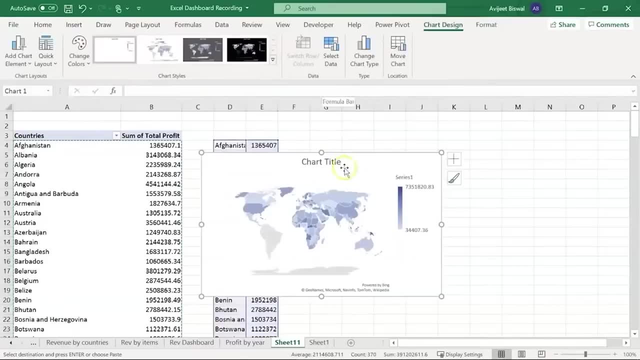 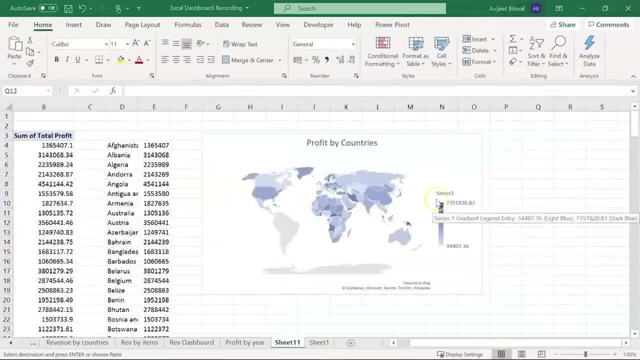 and i will paste it here. using this data, i can create my field map now, so i will go to insert here. we have the option to create a field map. there you go. you can see we have our map ready. i can expand this. as you can see, our map has a colour. 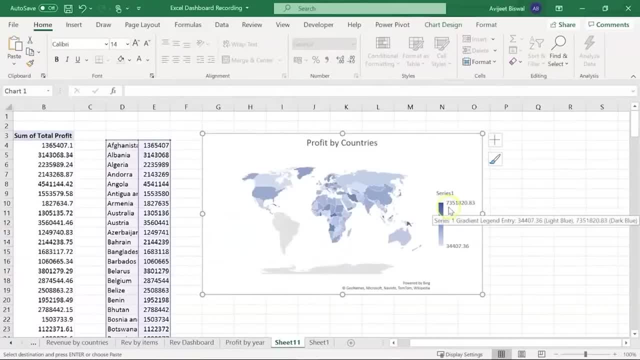 scale, which comes from light grey colour to dark blue colour. so the countries that are in grey or, you can say, light blue, have the lowest amount of profit, while the regions or the countries that have been shaded in dark colour or dark blue colour have highest amount of profit. 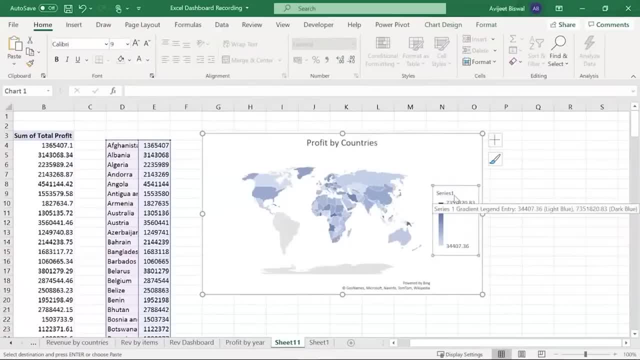 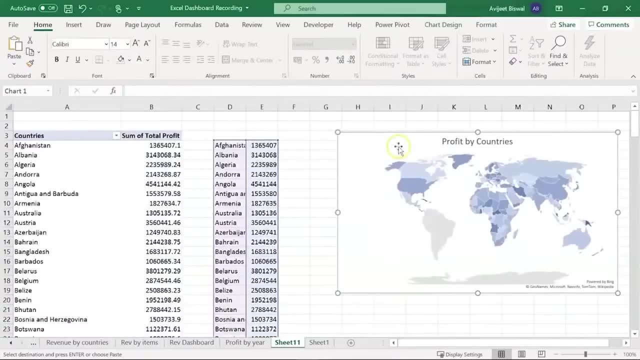 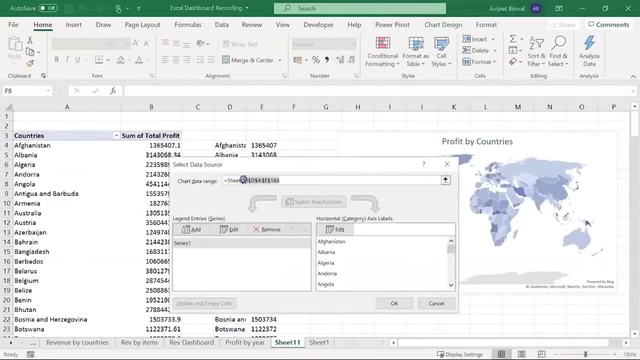 i will go ahead and delete this scale, ok. next we need to connect this map to the original data source. so what i will do is i will right click on this map and i will go to select data here. instead of the previous range, i will give my new range. 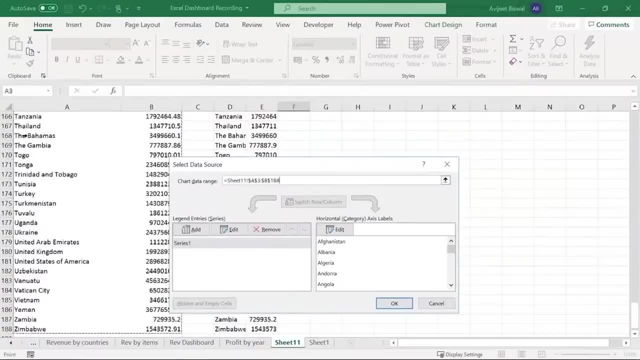 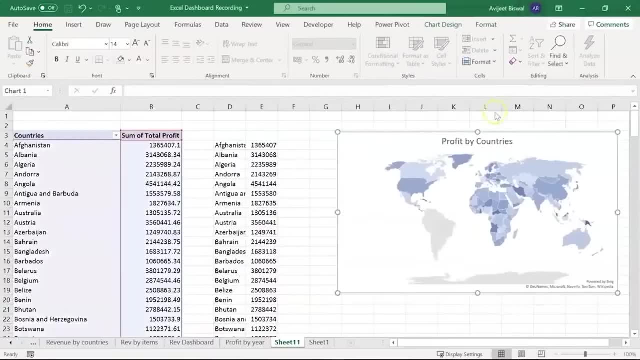 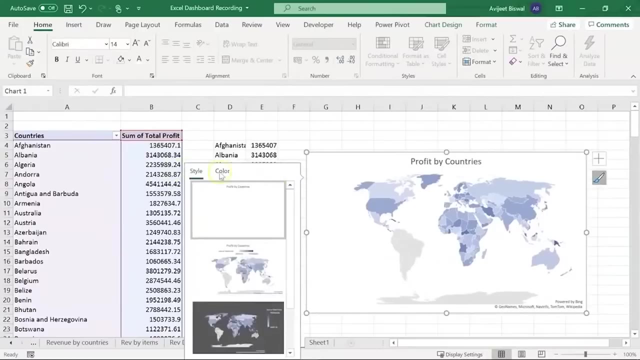 now. so my new range will be my original pivot table that i had created. go on top and click on ok. so we have our map ready now. now, if you want, you can change the colour of the shade. so i will just go to colours and lets say we will keep. 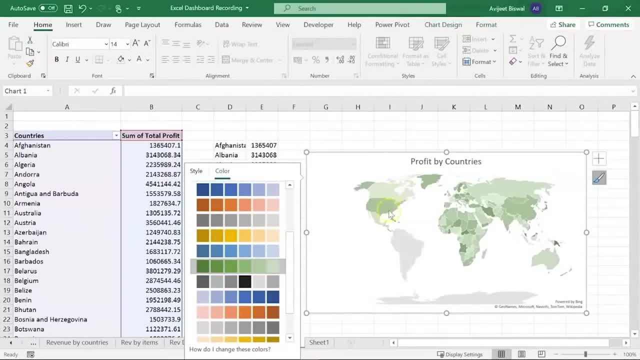 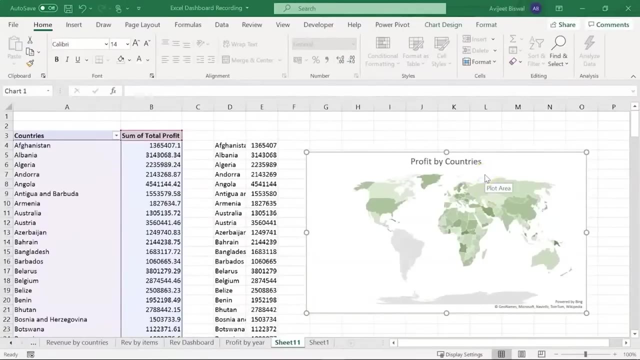 green colour. so the countries that are shaded in dark green have the highest amount of profit, while those which are highlighted in light green colour are the countries that made least amount of profit. ok, now, moving on. next, we want to create a pivot table that will show us the 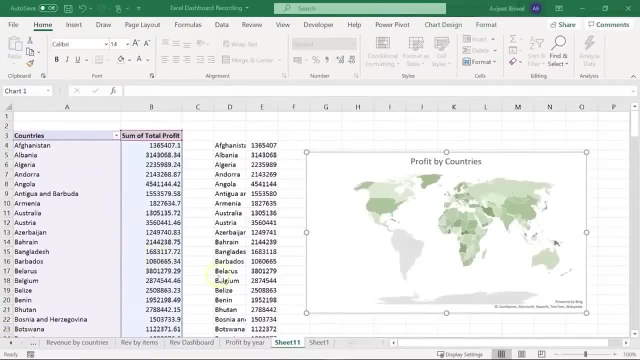 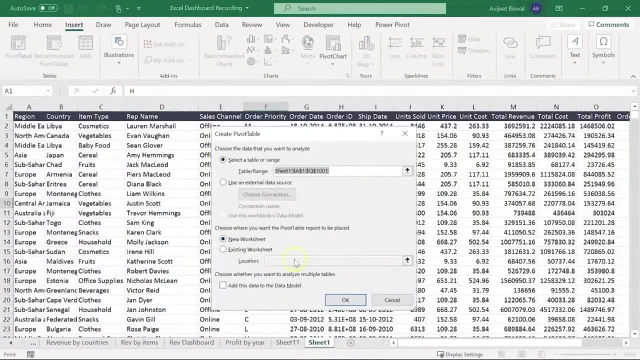 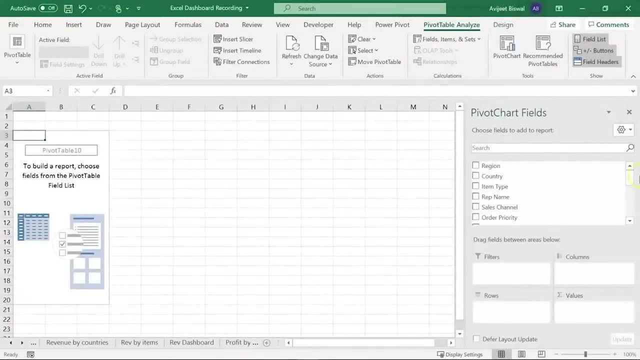 profit by year and sales channel. so for this we are going to create another line chart. so i will go to insert and click on pivot table. so i will select new worksheet here. since i want to know the profit by year first of all, i will drag my order year column. 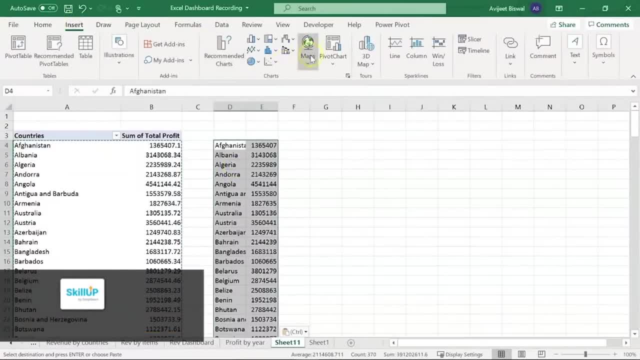 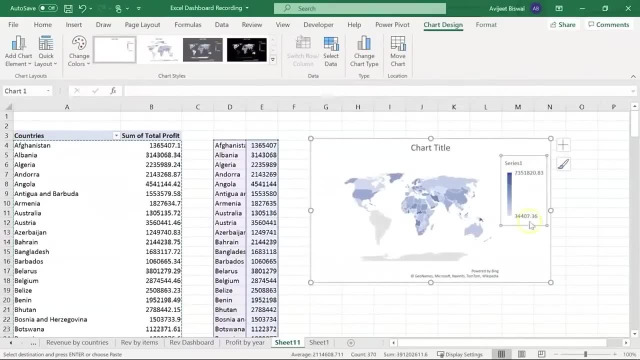 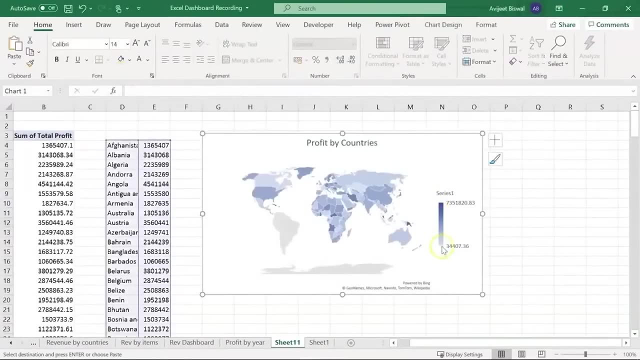 Now I Can Create My Field Map Now, So I'll Go To Insert Here. We Have The Option To Create A Field Map There You. 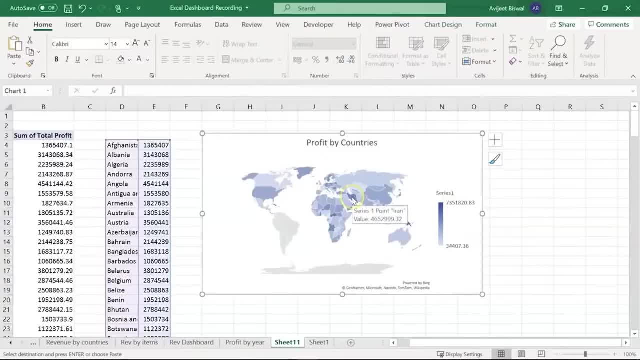 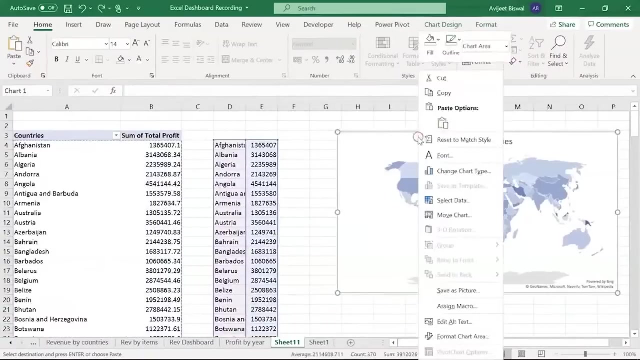 Go, You Can See That Shaded In Dark Color, A Dark Blue Color, Have Highest Amount Of Profit. I Will Go Ahead And Delete This. 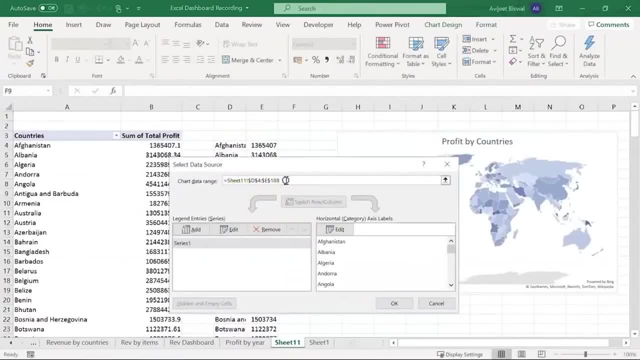 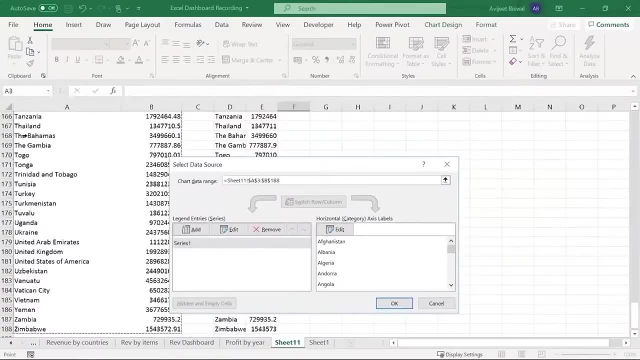 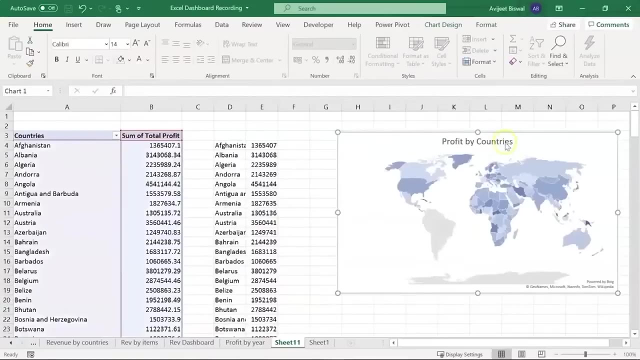 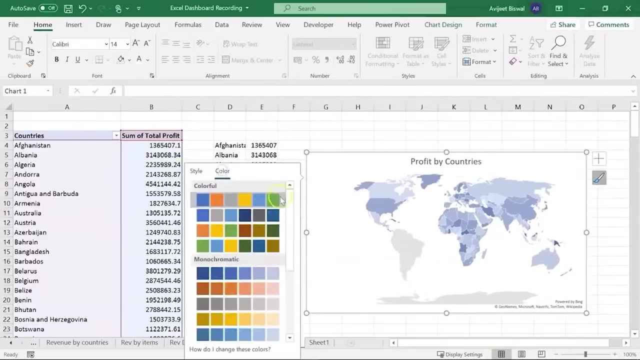 Scale. Okay, Next We Need To Connect This. My New Range Will Be My Original Pivot Table That I Had Created. Go On Top And Click. 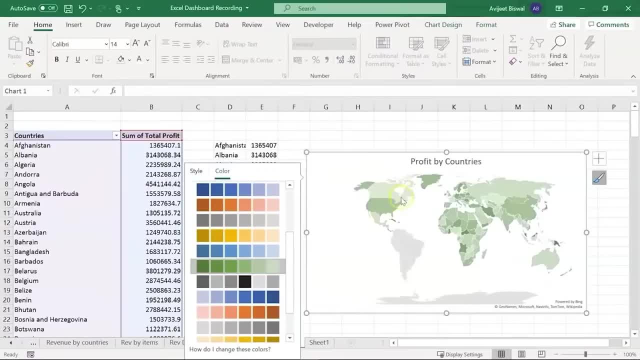 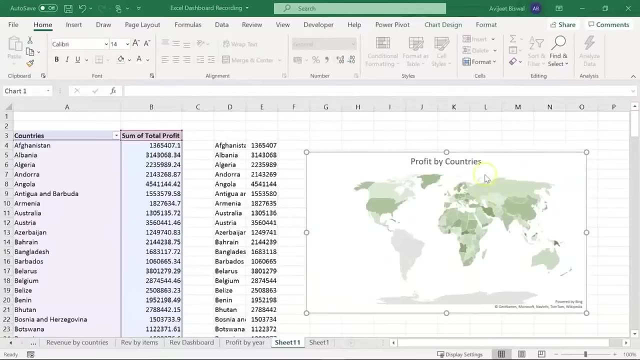 On. Okay, So We Have Our Map Ready Now. Now, If We Have A Light Green Color, Are Other Countries That Made Least Amount Of Profit. 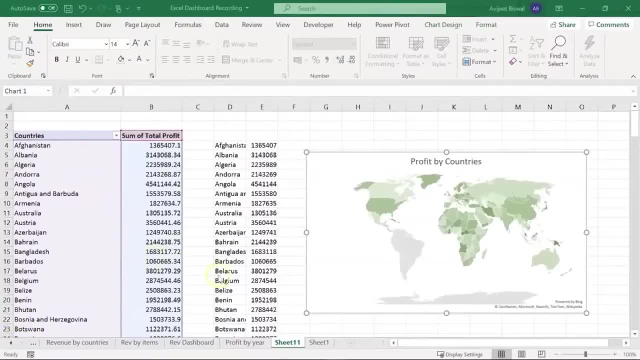 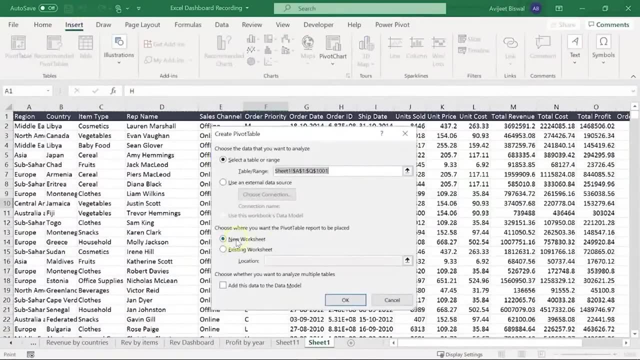 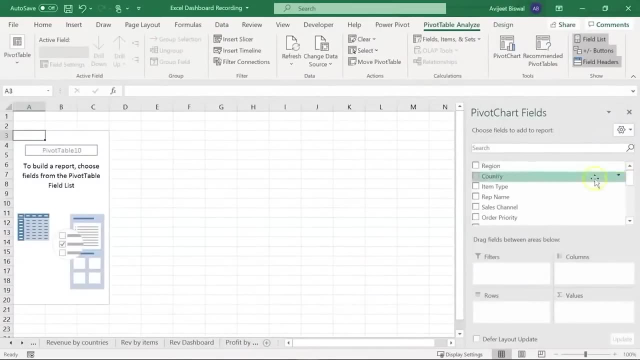 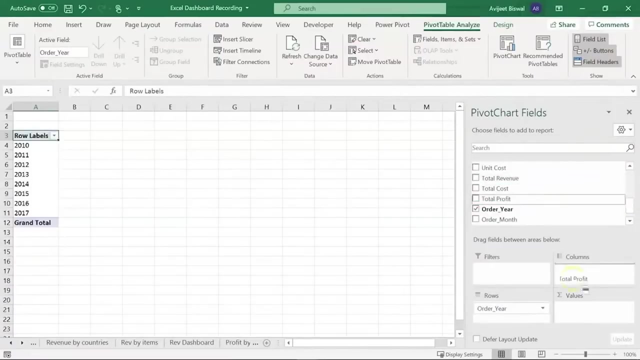 Okay, Now Moving On. Next, We Want To Create A Pivot Table That Will Work, Since I Want To Know The Profit By Year. First Of 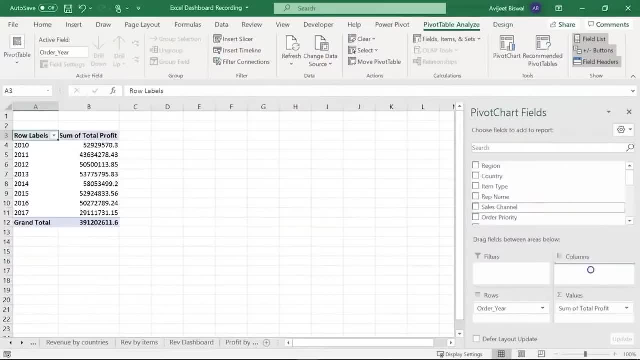 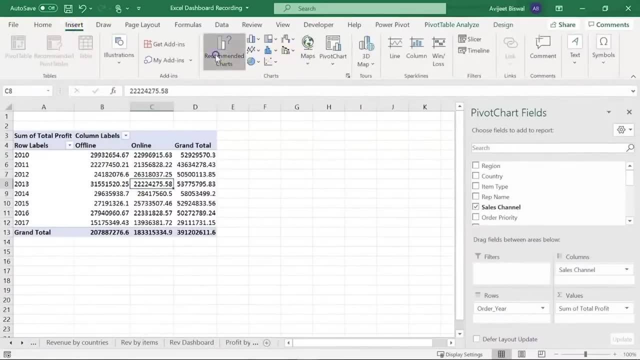 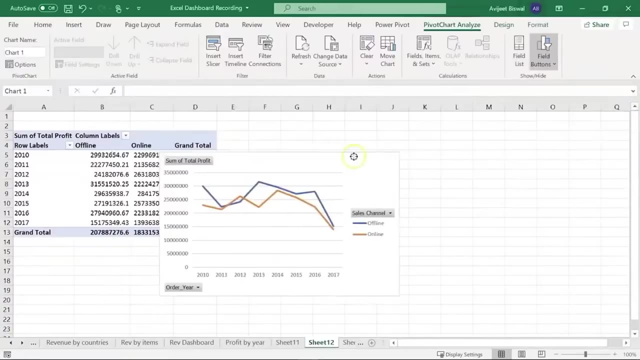 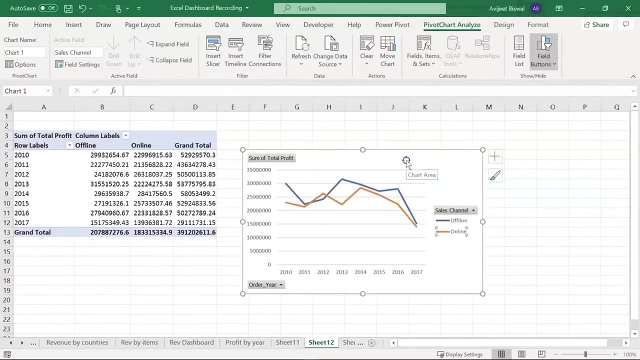 All. I'll Drag My Order Year Column To Rows And Then I'll Choose My Total Profit Column. This You See Here, Based On This Chart. 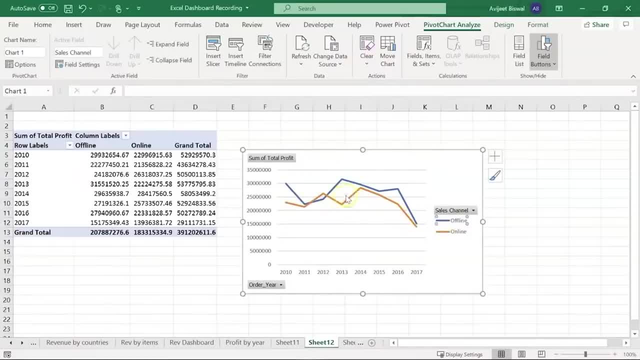 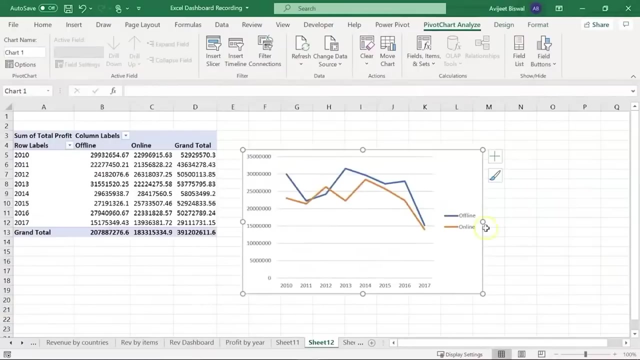 You Can Tell The Profit Generated With Online Sales Were Actually Lower Than That Of Offline. So Here The Blue Line. Let Me Go Ahead And 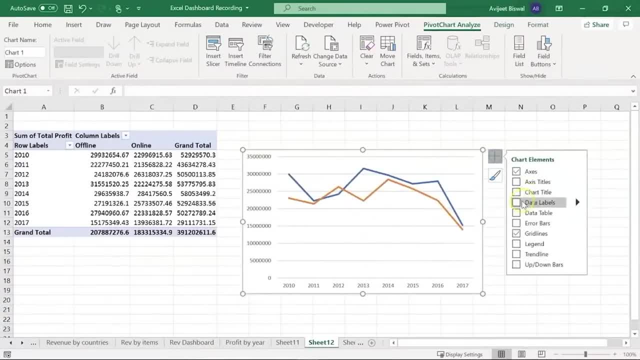 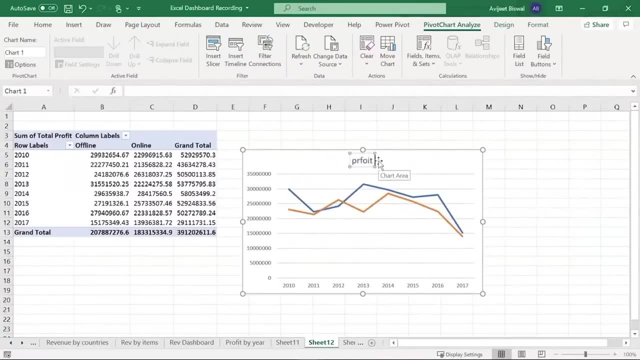 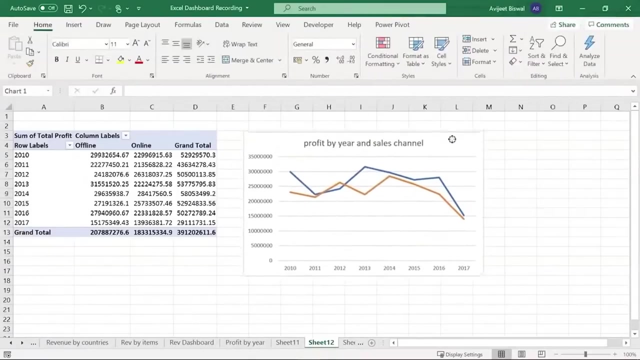 Edit This Chart A Bit, So We'll Delete The Field Buttons. I'll Also Delete The Legend. For Now, Let Me Go Ahead And Add My 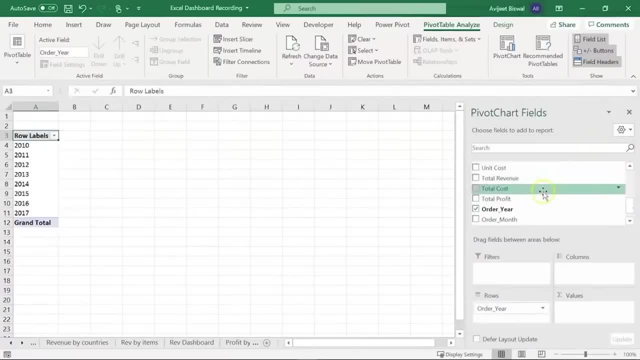 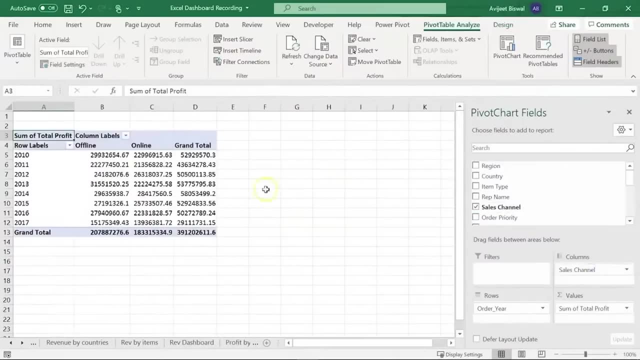 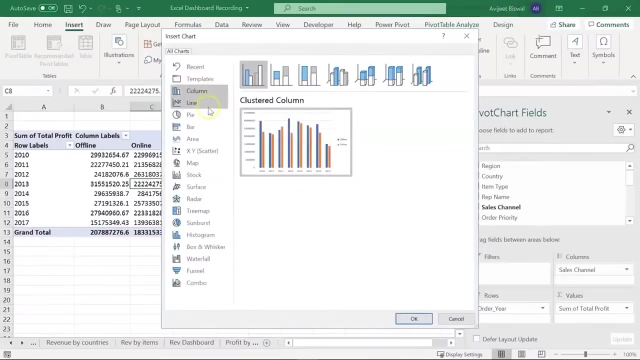 to rows and then i will choose my total profit column under values. next i am going to select my sales channel under columns. there you go. so we have our pivot table here. based on this pivot table, let me create my pivot chart. so i will go to recommended. 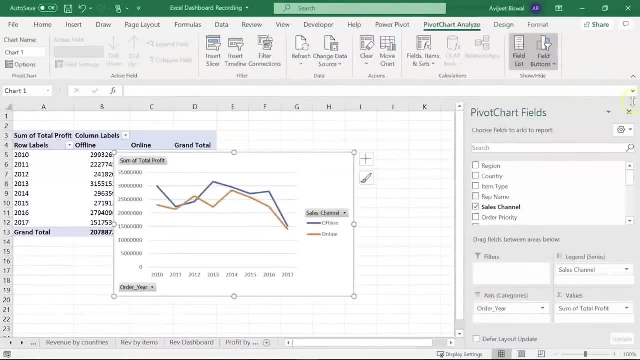 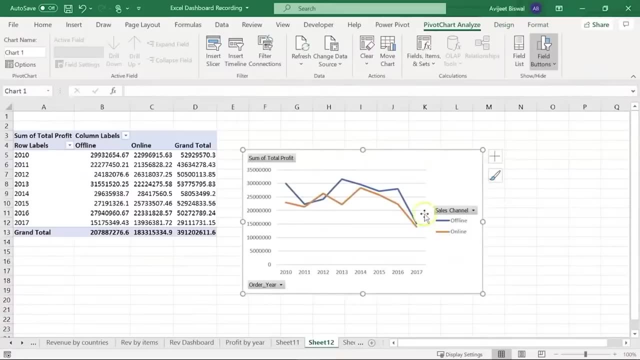 charts and i am going to create a line chart. i close this. you see, here, based on this chart, you can tell the profit generated with online sales were actually lower than that of offline. so here the blue line represents offline profit and the orange line represents online profit. 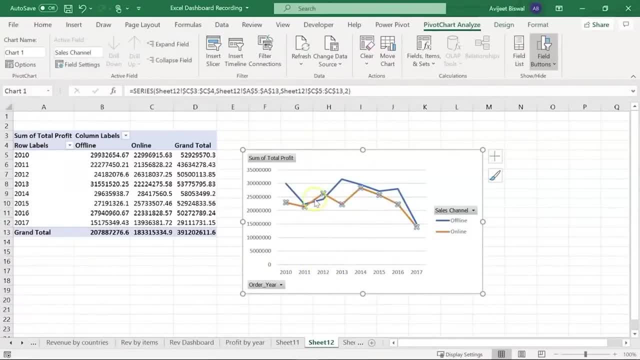 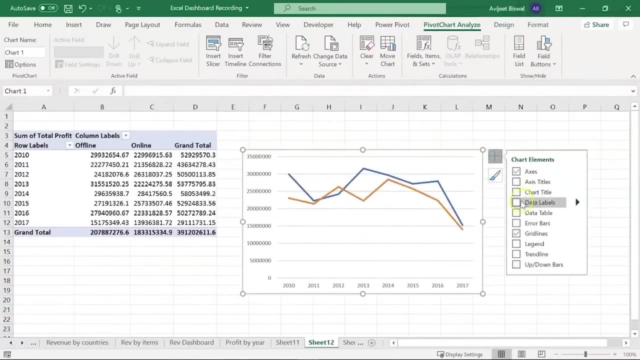 if you mark clearly, in year 2012 the online profit was actually higher than the offline profit. so let me go ahead and edit this chart a bit. so we will delete the field buttons. i will also delete the legend. for now, let me go ahead and add a chart title. 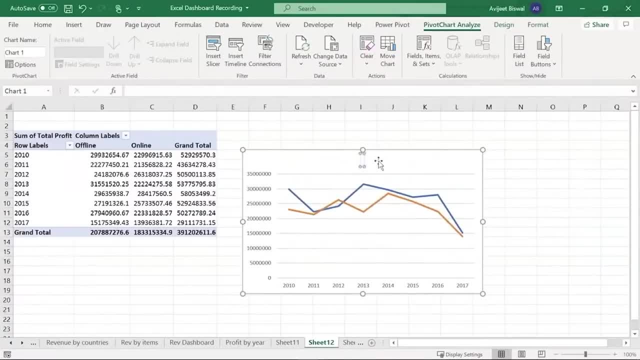 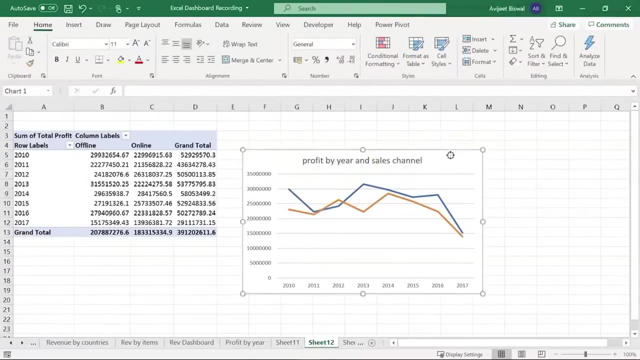 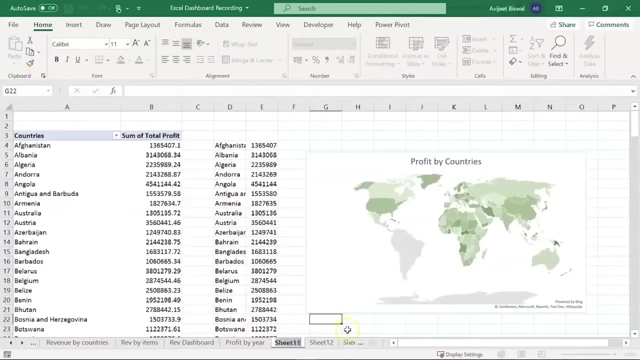 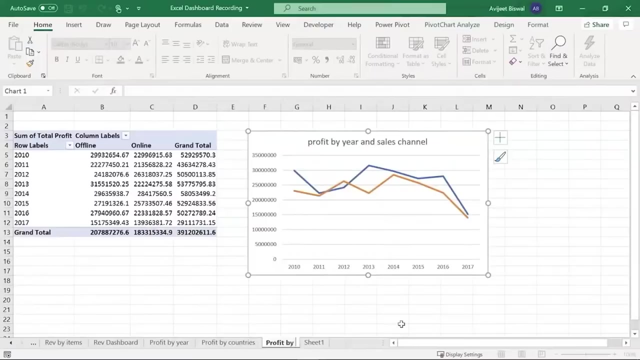 so i will write profit by year and sales channel. ok, so this is my second report before moving ahead. let me just rename this sheet, so i will write profit by countries. similarly, let me rename this sheet as profit by year and let's say sc for sales channel. ok, 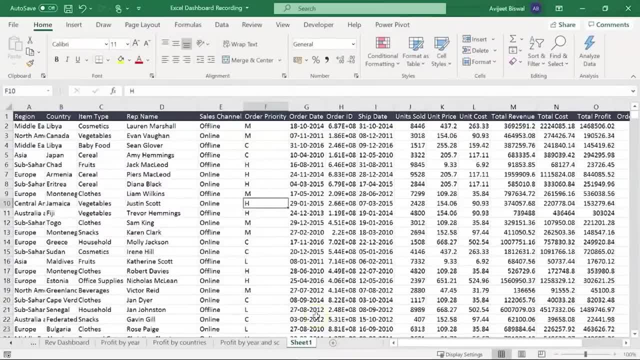 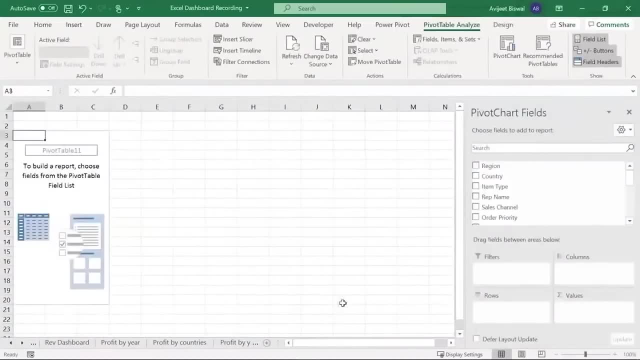 moving ahead now. i want to create a pie chart based on a pivot table that will show the profit by sales channel only. so this is going to be a simple pie chart, so i will first go to insert, click on pivot table and click on. ok, so i will drag. 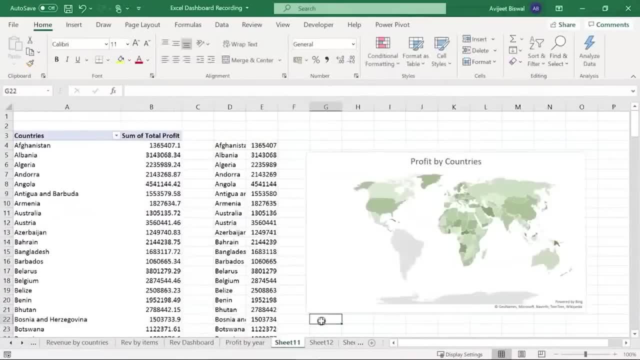 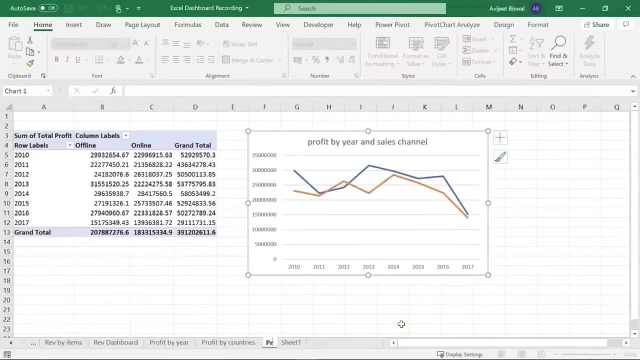 Second Report. Before Moving Ahead, Let Me Just Rename This Sheet, So I'll Write Profit By Countries. Similarly, Let Me Rename This Sheet As Profit. 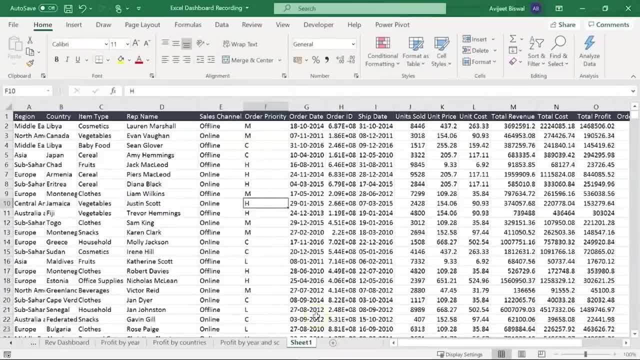 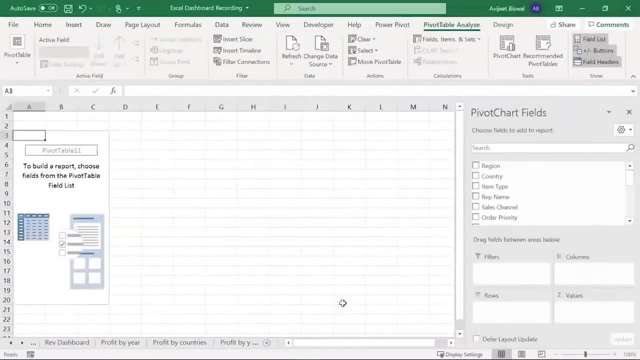 By Year And Value. Now I Want To Create A Pie Chart Based On A Pivot Table That Will Show The Profit By Sales Channel Only. 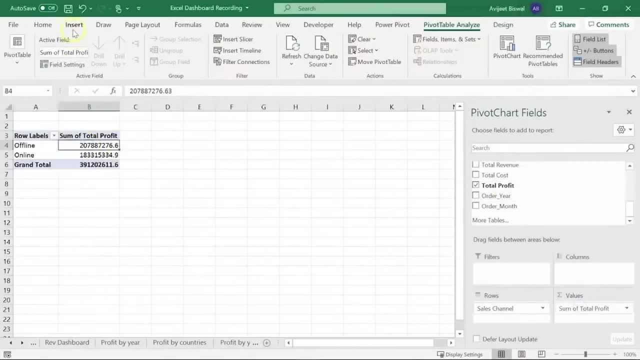 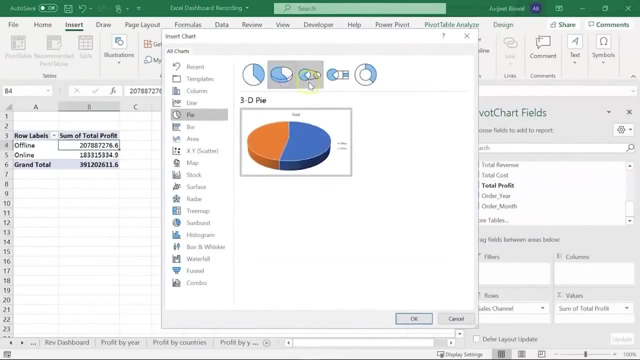 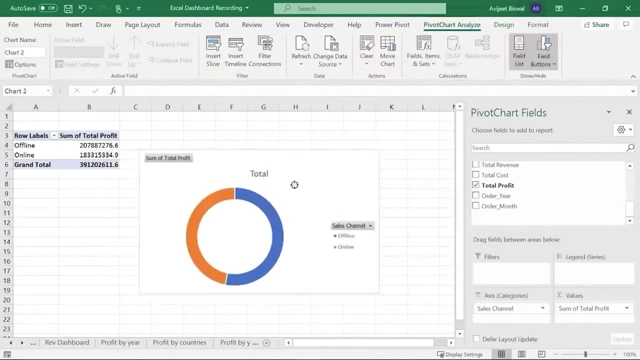 So This Is Going To Be A Pivot Chart, Which Is Going To Be A Pie Chart. Let Me Explore The Other Types Of Pie Charts. 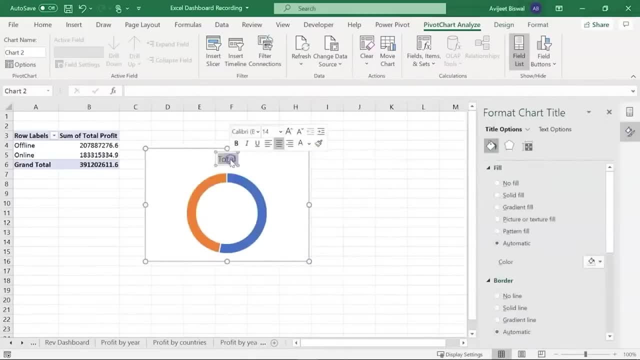 We Have. Okay, So I'm Going To Select A Sales Channel. Okay, Let's Also Add Data Labels, And Here Again I'm Going To Format. 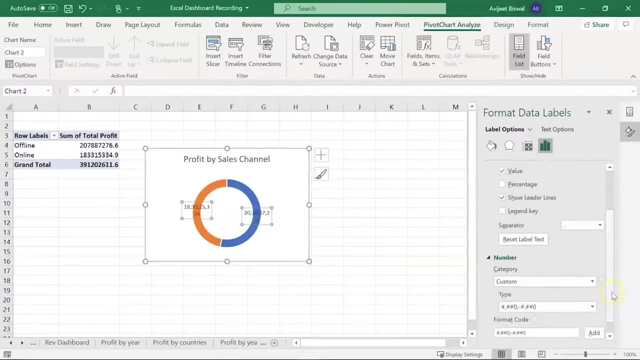 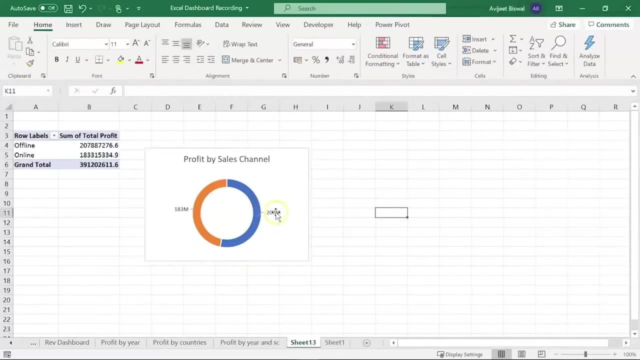 This Label. I'll Select The Category As Custom And My Type To The Left And This To The Right. Okay, Let's Also Delete The Lines. 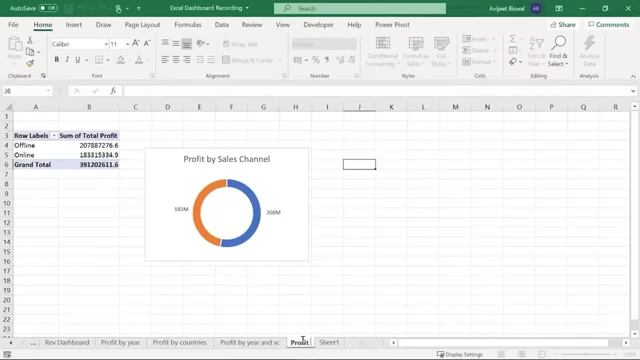 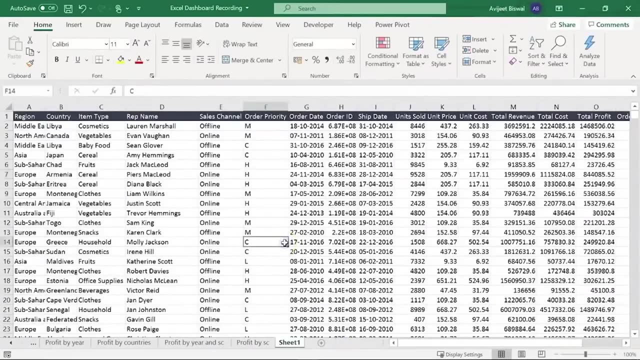 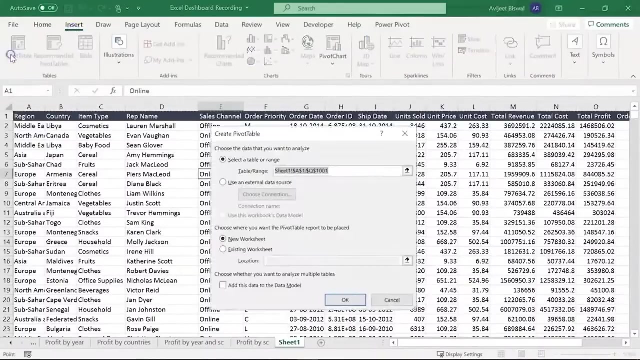 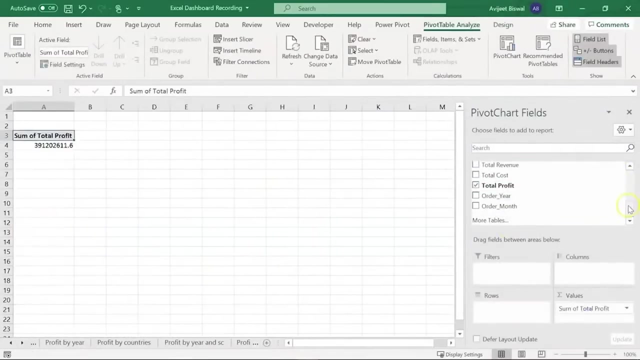 Cool, Now Let Me Just Rename This Sheet So I'll Write Profit By. Let's See Which Go Ahead And Create My Pivot Table First This: 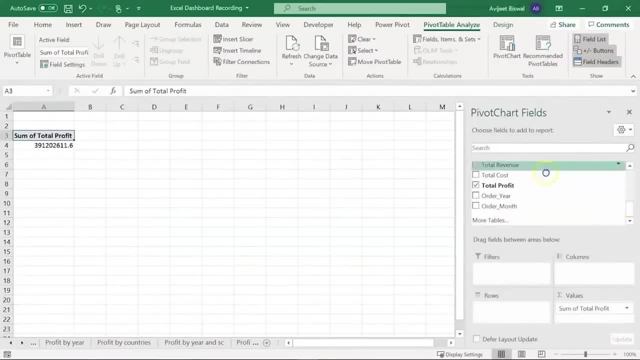 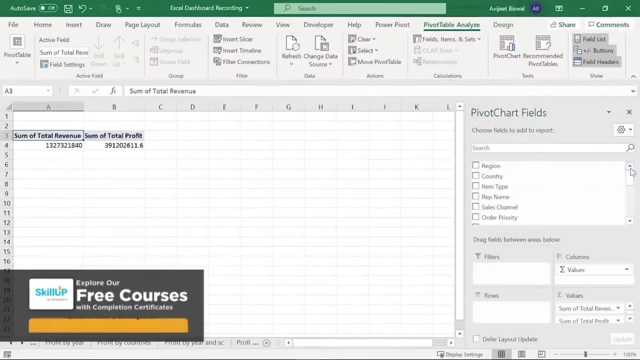 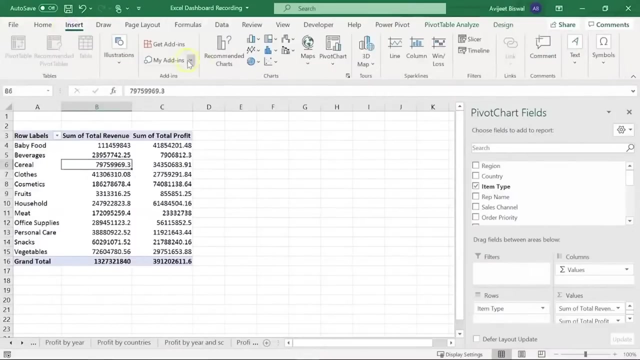 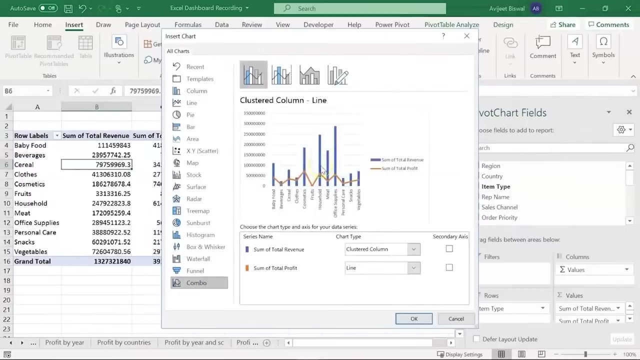 Time I'll Choose My Total Profit Under Values And Will Also Have The Revenue Column, So I'll Put My Revenue At The Chart, So You 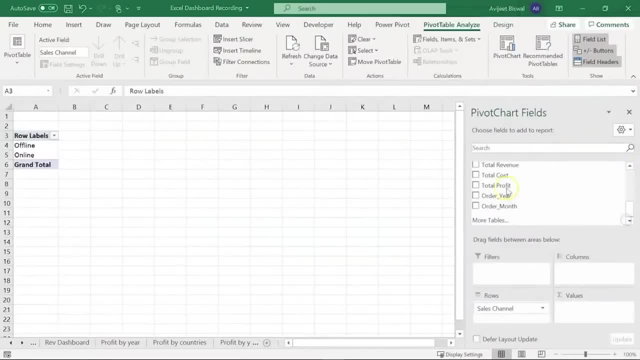 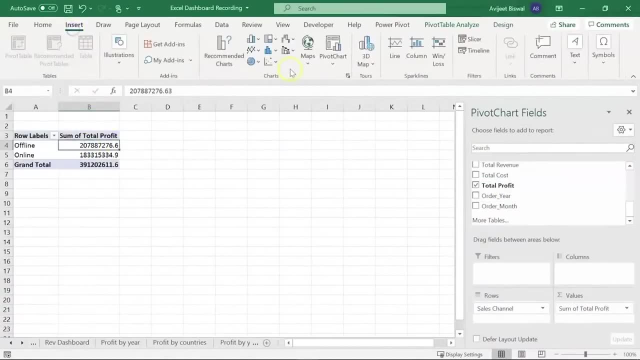 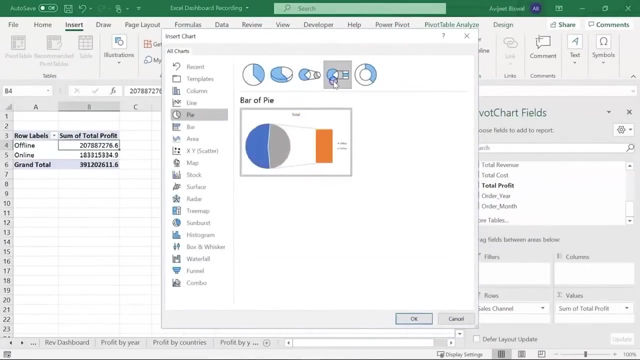 my sales channel under rows and then we will have the total profit column under values. so this is my simple pivot table. now let's create our pivot chart, which is going to be a pie chart. let me explore the other types of pie charts we have. ok, so i am going to select a donut chart. 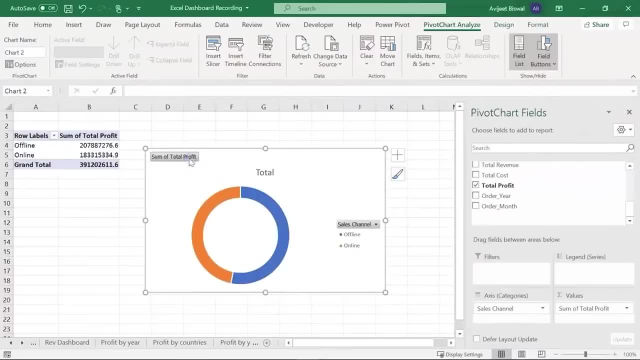 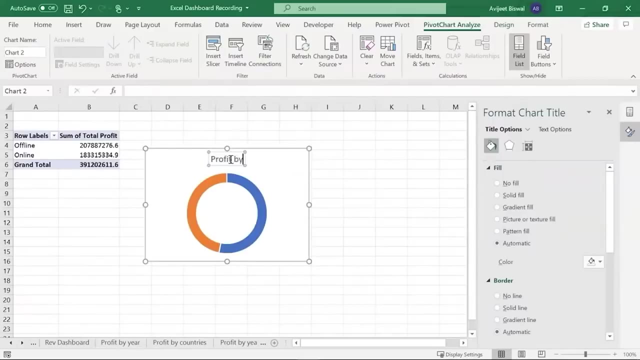 here and click on: ok, let's edit this chart. i will remove the field buttons. let me now remove the legend as well. i will just resize it. and this is going to be profit by sales channel. ok, so let's also add data labels. and here again i am. 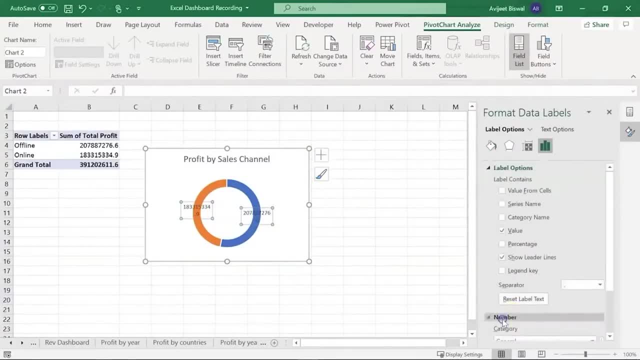 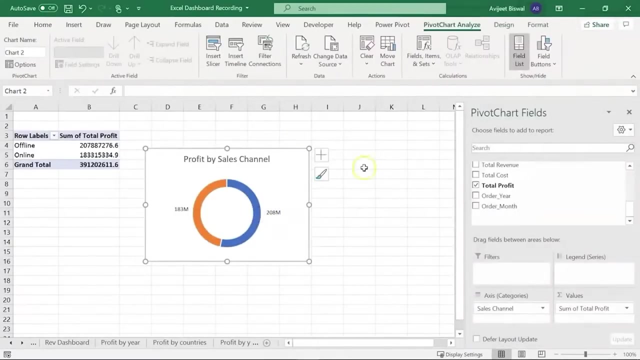 going to format this label. i will select the category as custom and my type will be in millions. ok, let me just move this to the left and this to the right, ok. ok, let's also delete the lines. cool, now let me just rename this sheet, so i will write. 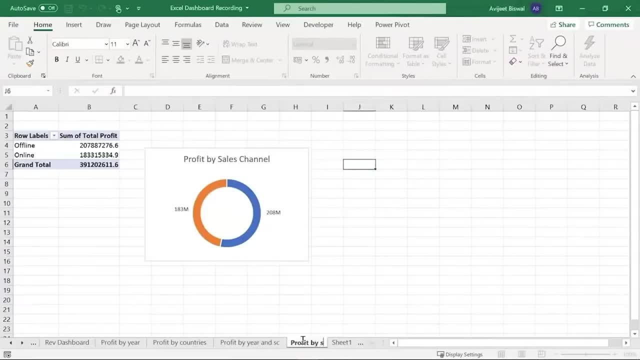 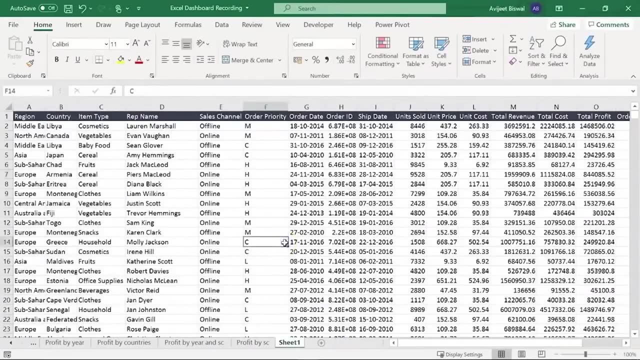 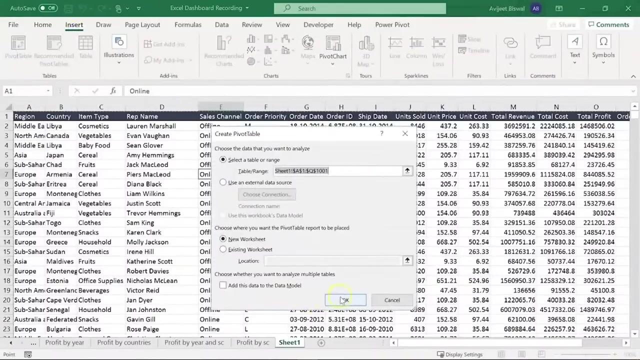 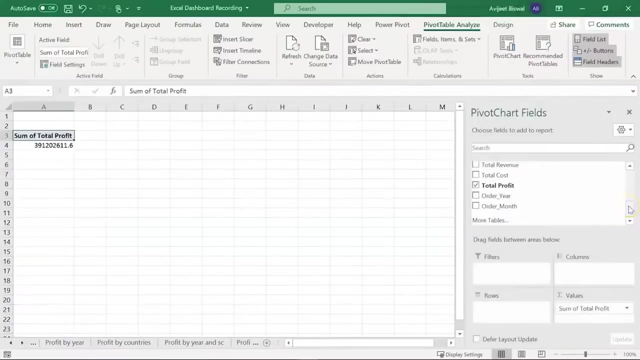 profit by, let's say, sc, which stands for sales channel- cool. finally, i am going to create a report that will show the revenue and profit by items, so i will go ahead and create my pivot table first. this time i will choose my total profit under values, and we will also have 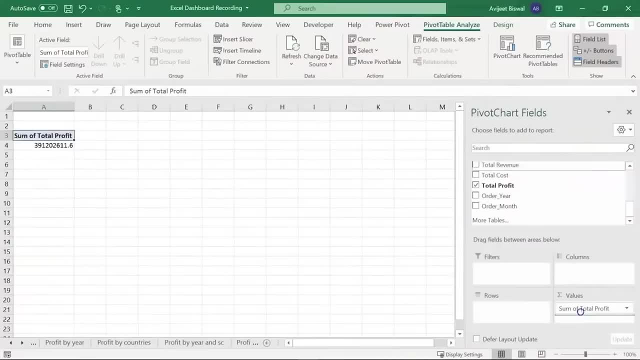 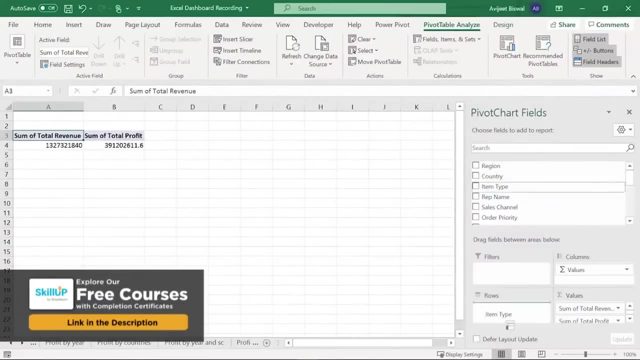 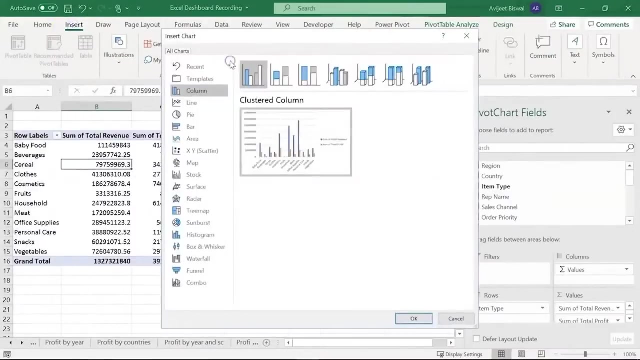 the revenue column, so i will put my revenue at the top. then i am going to select item type under rows. so here is my pivot table. based on this pivot table, let me now create a combo chart. so you can see the preview of the chart the blue bars represent. 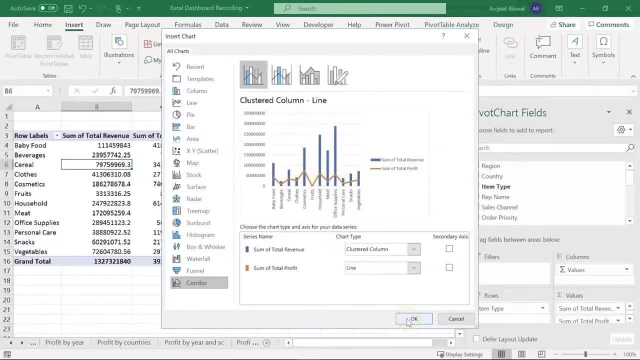 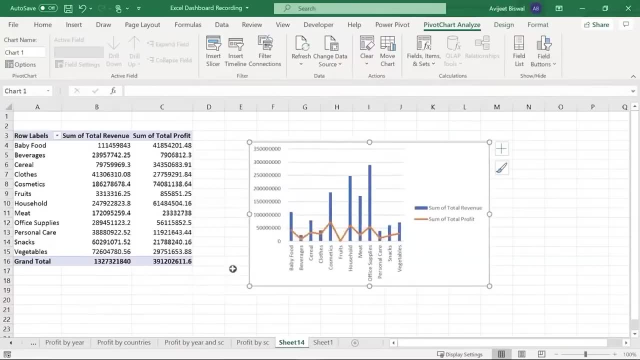 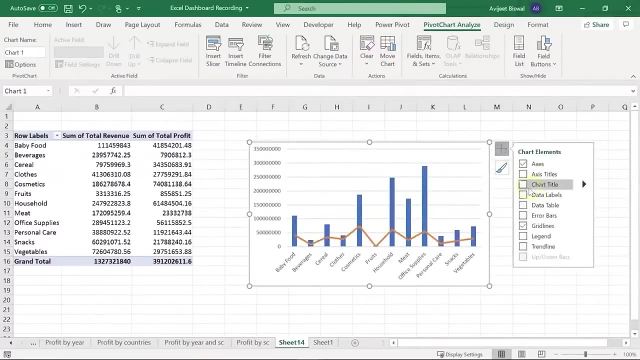 the total revenue and the orange line represents the total profit i will click on. ok, let me close this. first, let's remove the field buttons. let's also remove the legend here. then we will add a chart title. i will name it as revenue and profit by items. 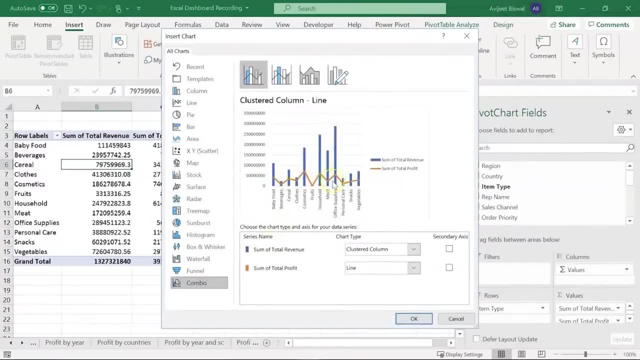 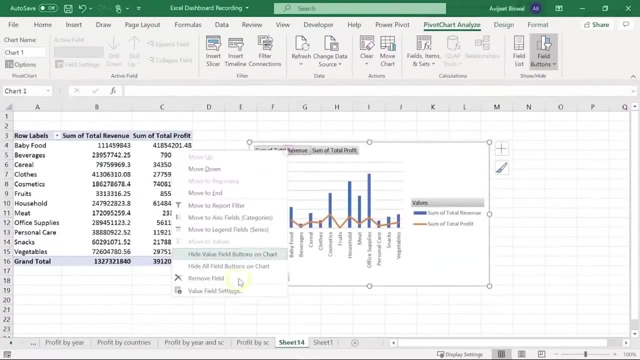 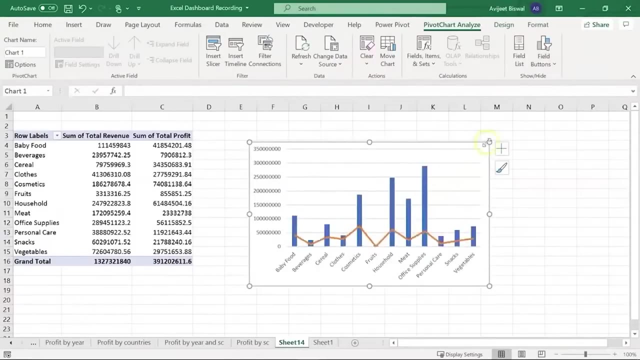 Can See The Preview Of The Chart. The Blue Bars Represent The Total Revenue And The Orange Line Represents The Total Profit. Click On Okay, So. 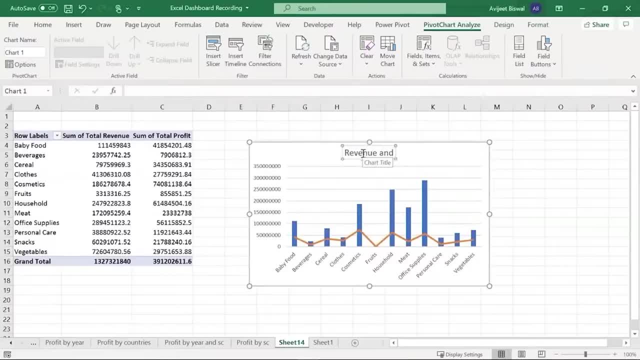 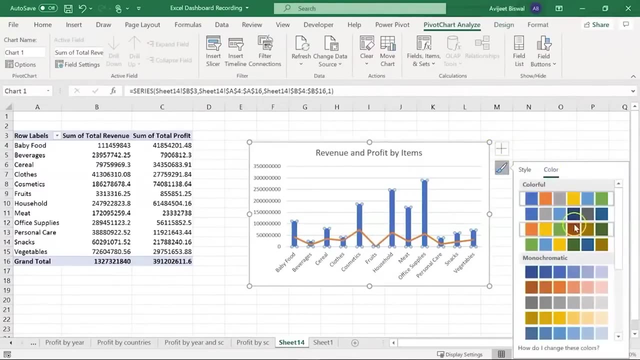 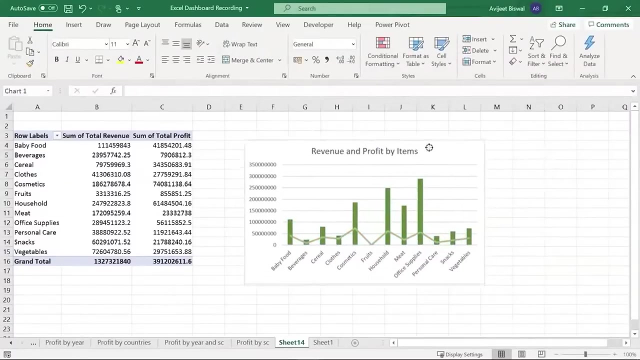 We Have The Total Revenue And Profit By Items. Okay, If You Want, You Can Also Go Ahead And Change The Color Of The Bars. So 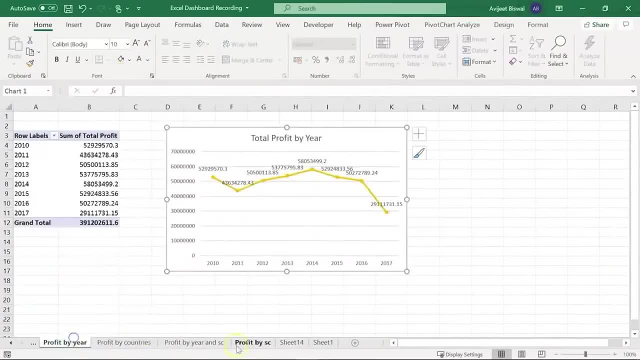 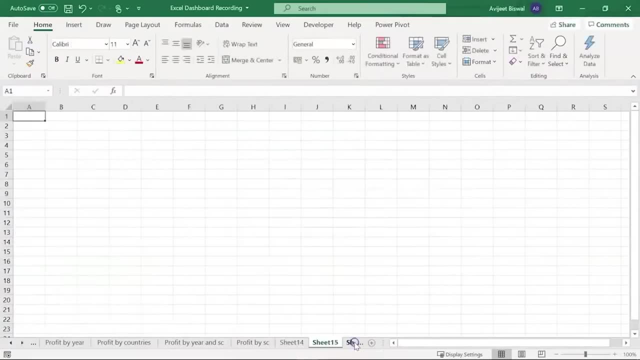 Let Me Just Create Our Profit Dashboard. Next, Let's Create A New Sheet And We'll Get Started With Building Our Dashboard. So I'll Click. 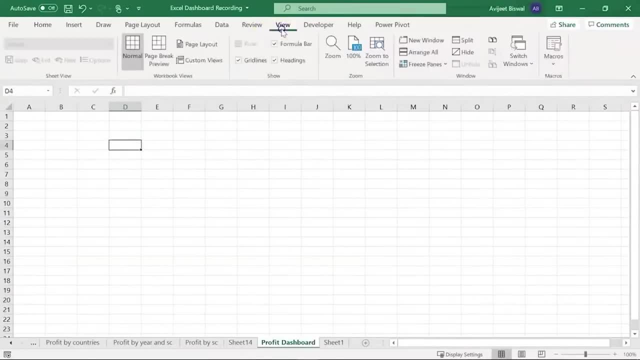 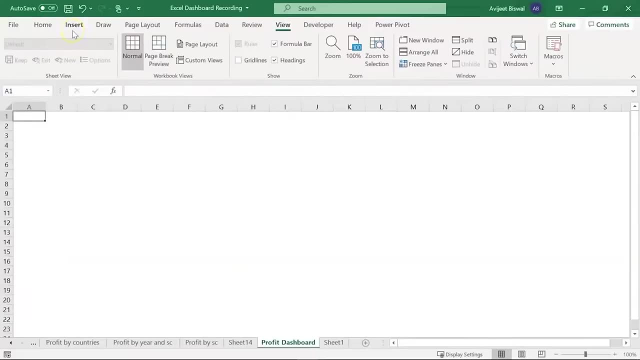 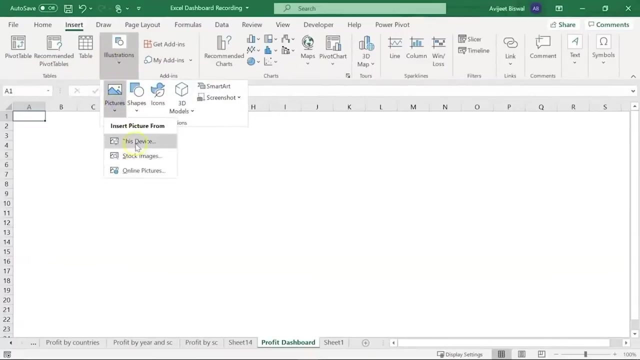 On A New Sheet, Let Me Just Rename. We'll Insert A Background Image, Like We Did For Our Revenue Dashboard, So I'll Go To Insert. 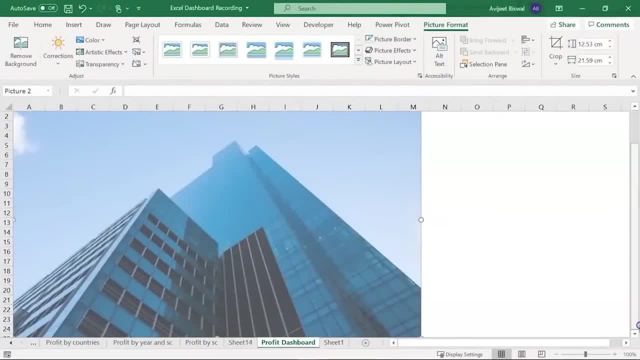 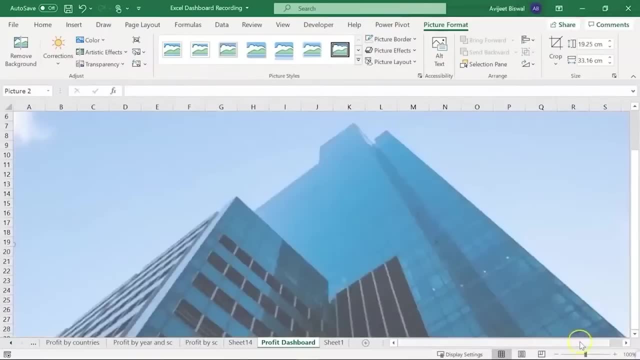 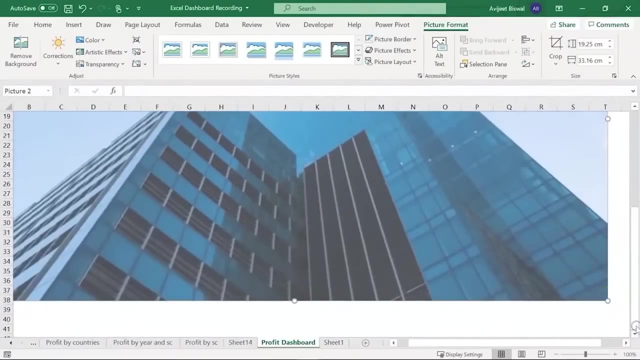 Under Illustrations. I'll Click On Pictures And Select This Device. I'm Going To My Revenue Dashboard. We'll Adjust The Size Also. All Right Now. 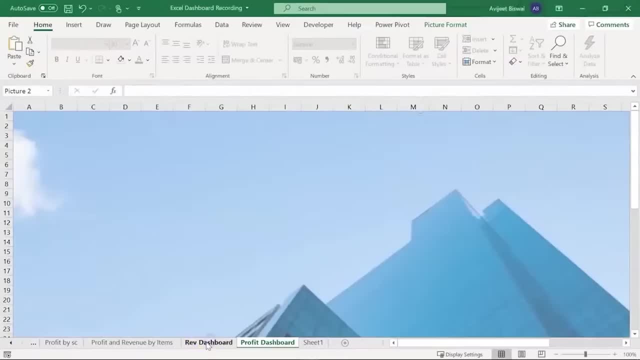 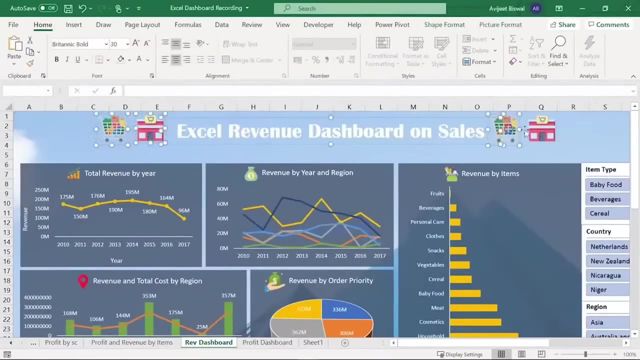 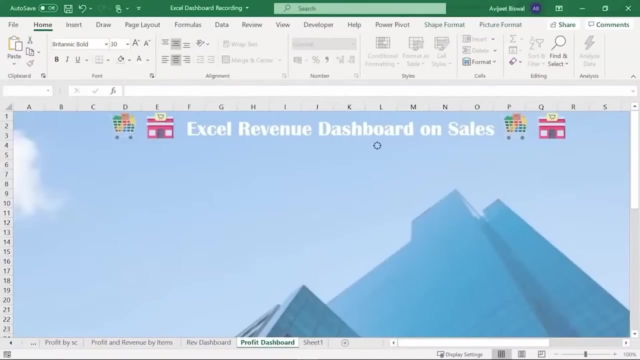 Let's Copy The Title Of My Profit Dashboard. So Here You Can See I Have Brought My Revenue Dashboard In The Center. All Right, The 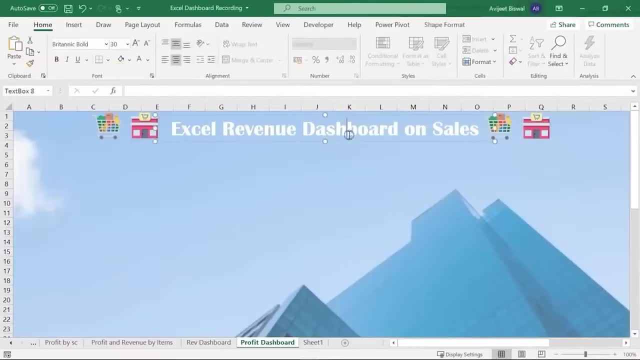 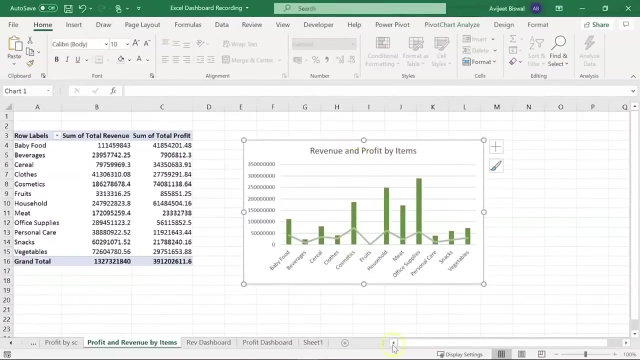 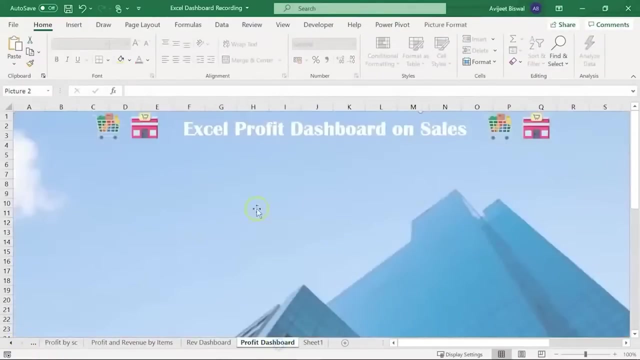 Next Step. Let Me Now Go Ahead And Edit The Title. So This Is Actually Going To Be Excel Profit Dashboard Instead Of The Profit Dashboard. 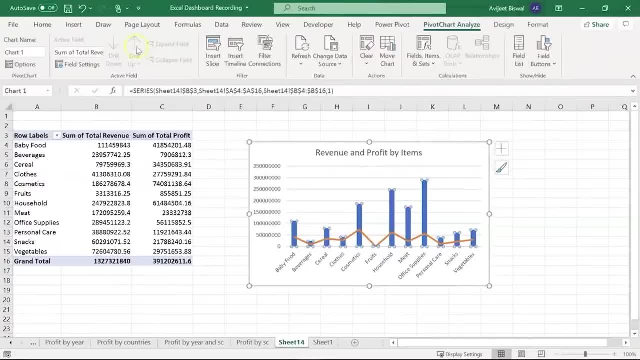 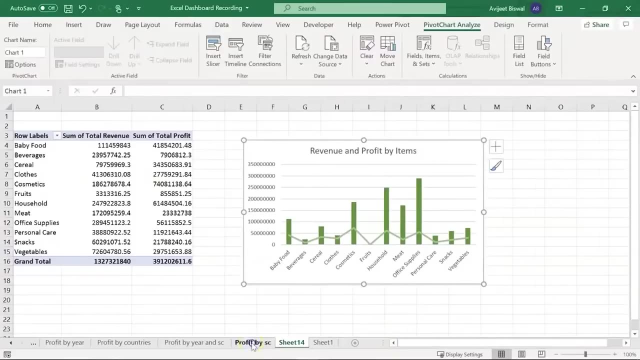 ok, if you want, you can also go ahead and change the color of the bars, so let me just select one of these colors. ok, alright, so we have our five reports ready that we are going to use for our profit dashboard. next, let's create a new sheet. 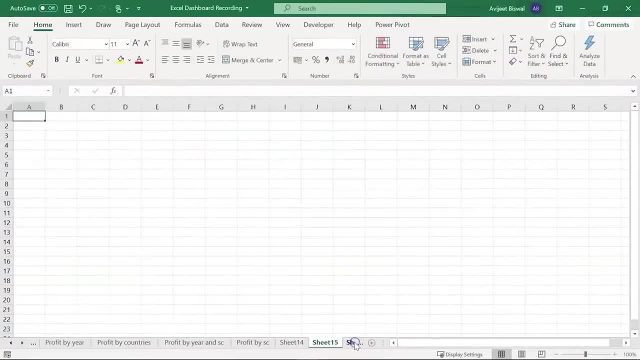 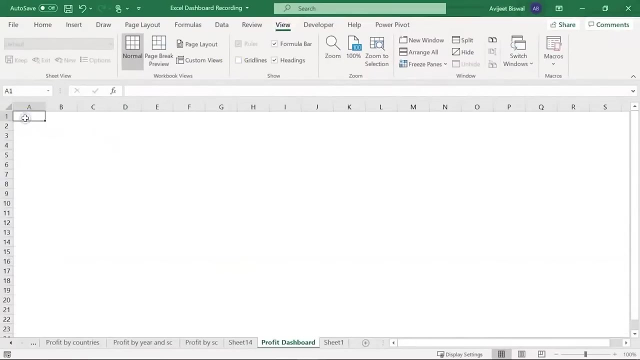 and we will get started with building our dashboard. so i will click on a new sheet. let me just rename this as profit dashboard. alright, we will continue with the previous drill. so first of all, let's go to the view tab and remove the grid lines. now we will insert. 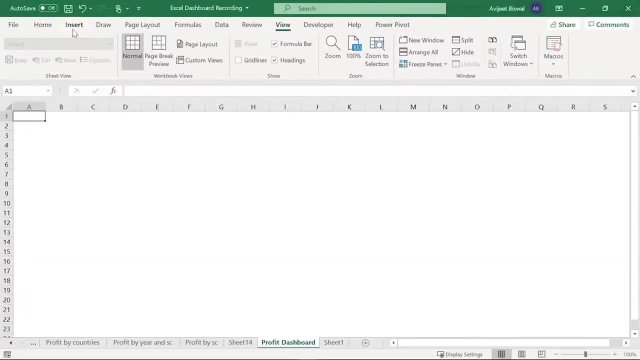 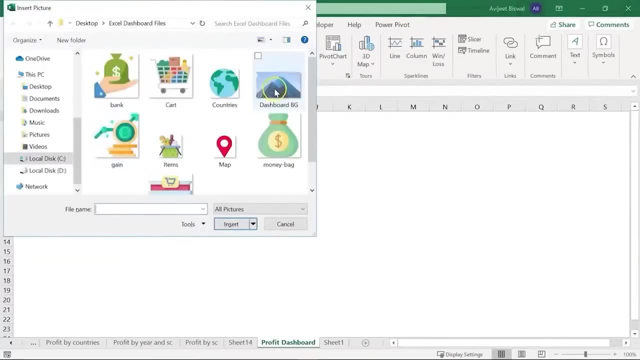 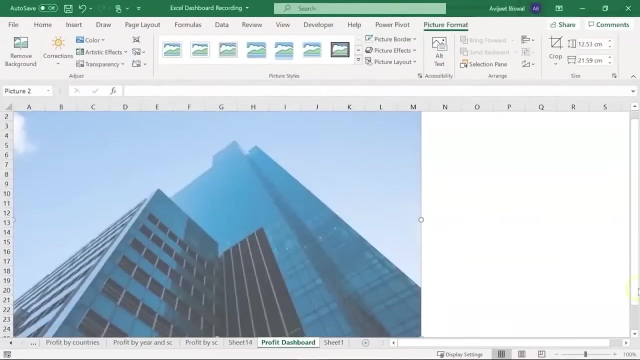 a background image, like we did for our revenue dashboard. so i will go to insert under illustrations. i will click on insert and select this device. i am going to have the same background. i will click on insert. alright, so you can see. we have a picture of a. 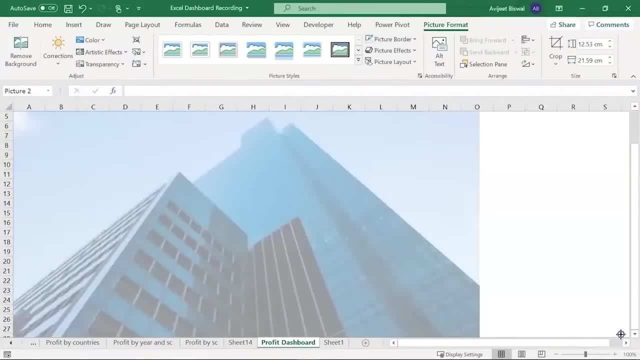 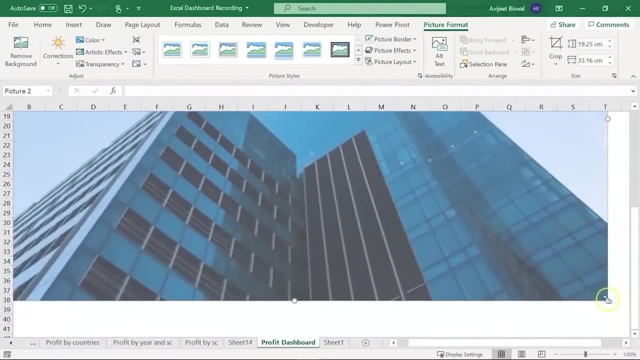 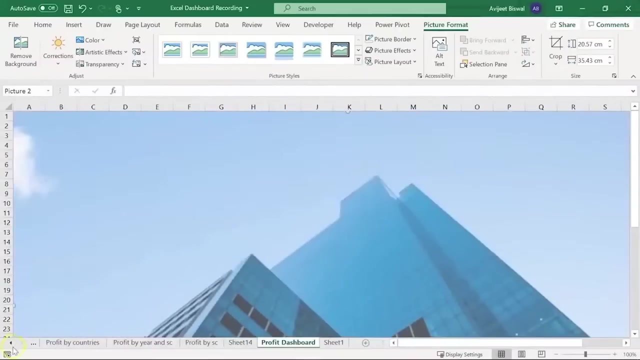 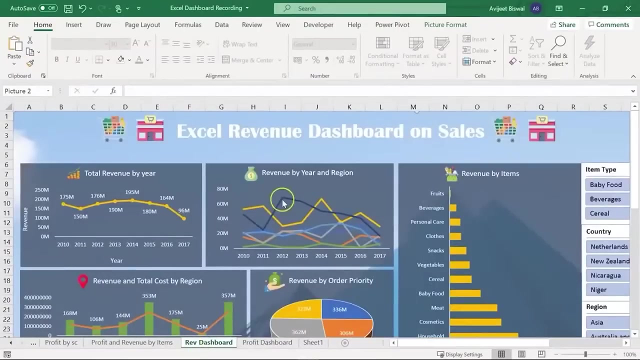 company, or you can say an organization. let's just drag this a bit to the right. we will adjust the size also. alright, ok, now let's copy the title of my profit dashboard. so here you can see i have brought my revenue dashboard and i will copy the title and the logos. 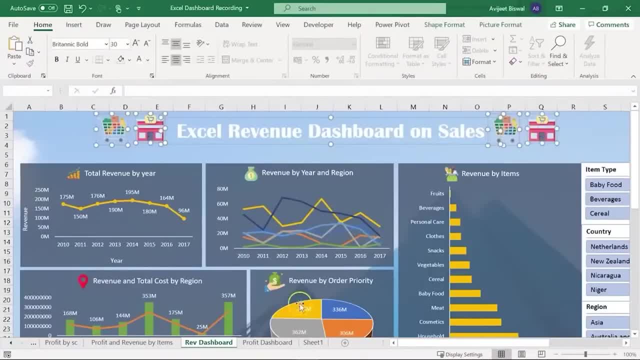 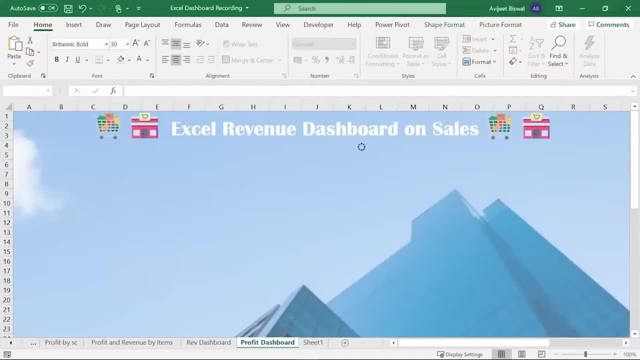 that we used for the revenue dashboard. i will paste it on my new dashboard. let's just align it in the center. alright, the next step. let me now go ahead and edit the title, so this is actually going to be excel profit dashboard instead of revenue. now we will copy each of the charts that. 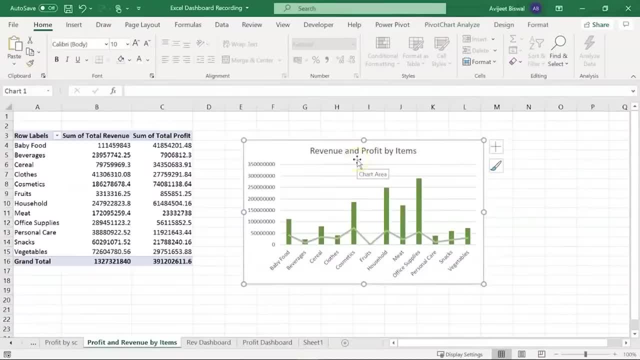 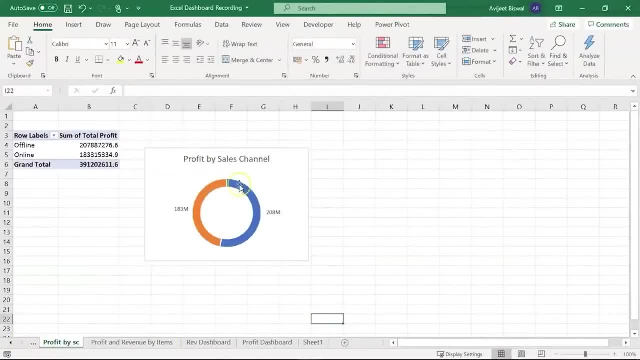 we just created, for example, the revenue and profit by items, then we had profit by sales channel. all this we are going to copy one by one and put it on the profit dashboard. so let me just copy a few now. i will paste it here and later on we can make the adjustment. 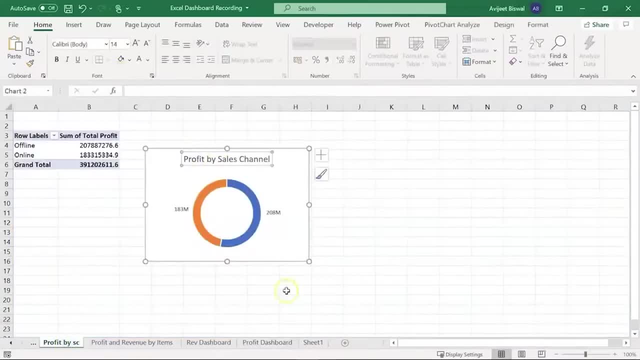 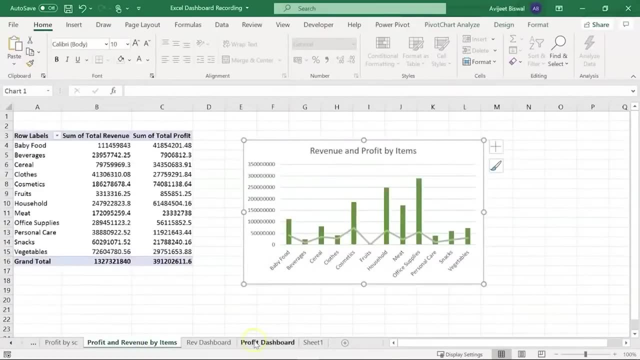 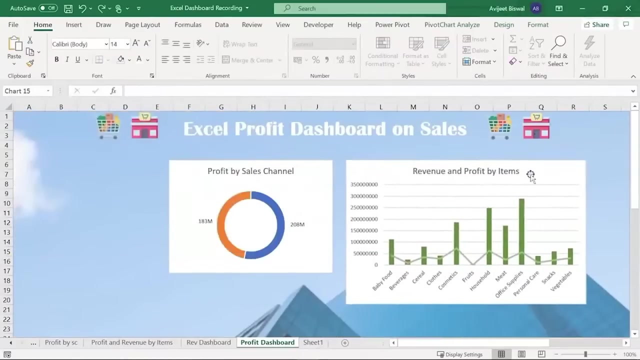 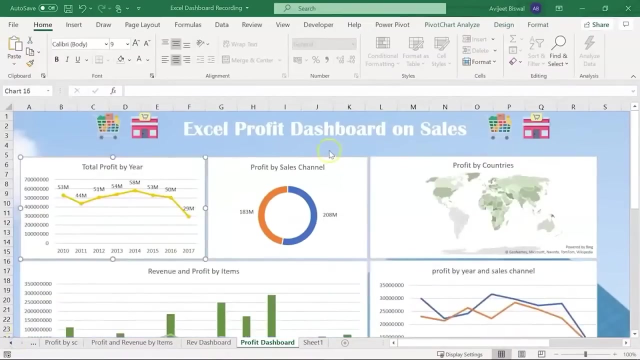 So Let Me Just Copy A Few Now. I'll Paste It Here, And Later On We Can Make The Adjustment. Copy This As Well. Similarly, 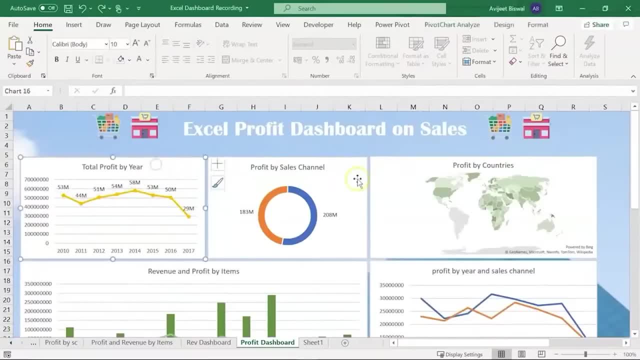 I'll Make The Profit Dashboard. I've Added All The Charts And I've Aligned And Reshaped It So That It Looks Good. I've 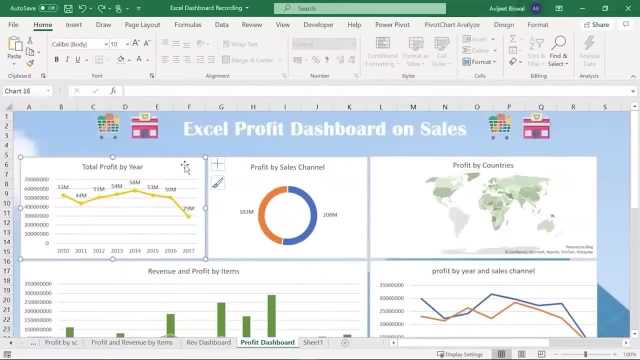 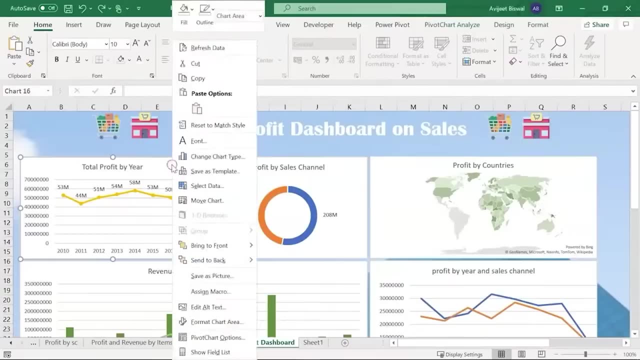 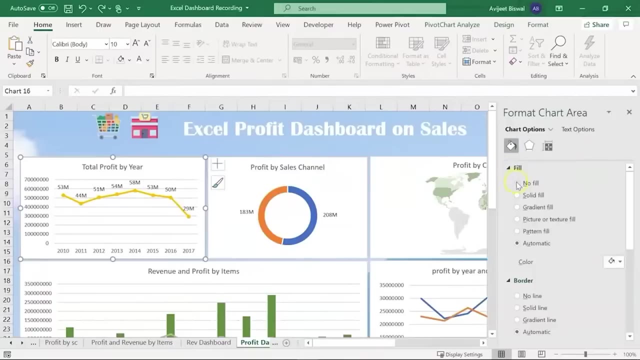 Also Made Some Formatting. For Example, I've Reduced Select The First Chart. I'll Right Click And I'll Click On Format Chart Area Here Under. 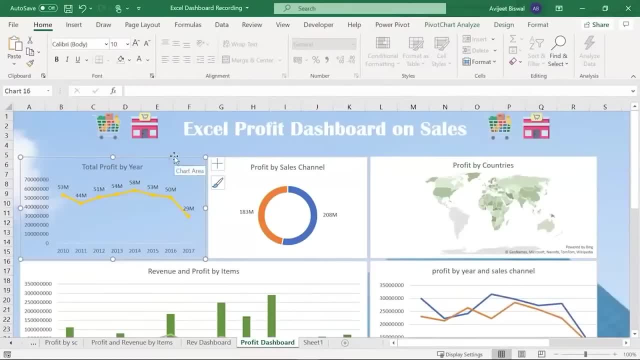 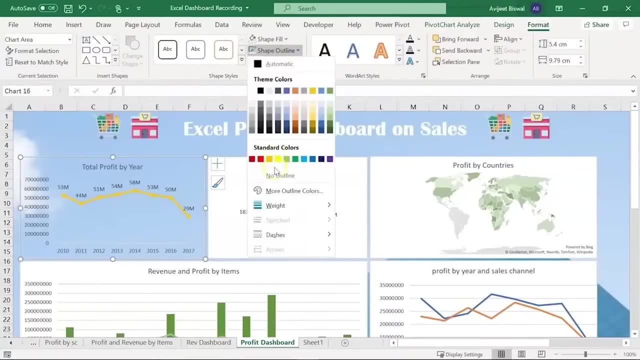 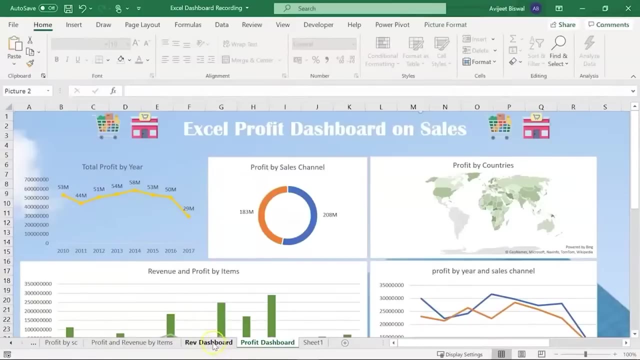 Fill. I'll Select No Fill. Next, I'm Going To Remove The Gridline, So I'll Going To Add A Blue Box At The Back, Like. 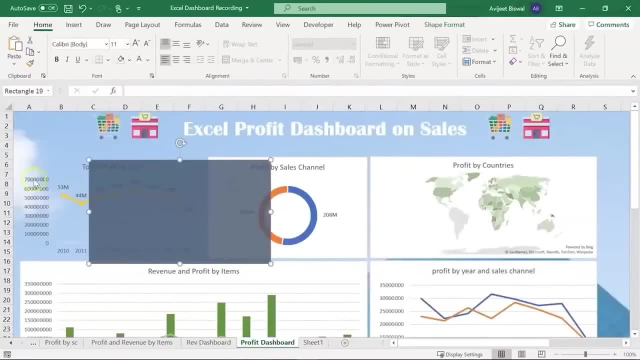 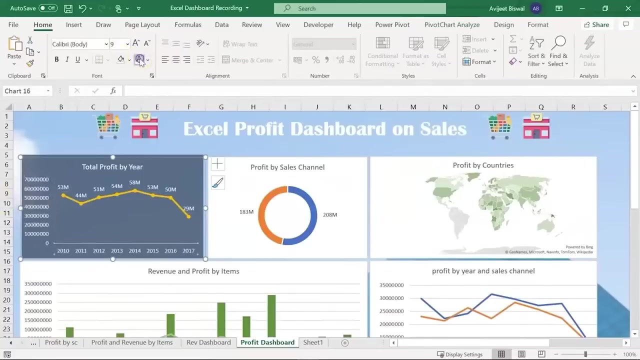 How We Did For The Revenue Dashboard. So Let Me Select A Blue Box From Here, And I'm Going To Format The Chart, So I'll. 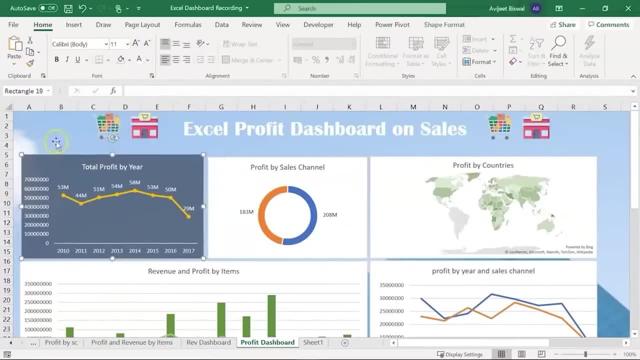 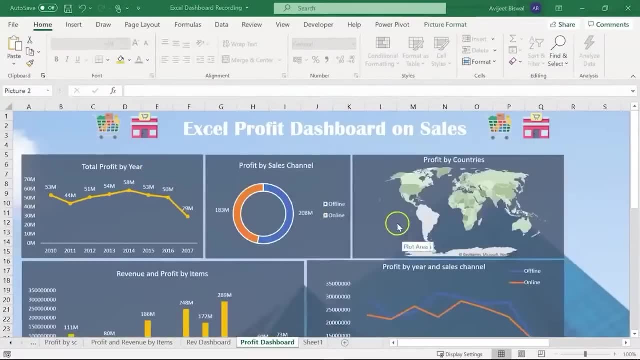 Click On Format The Chart. So Here I'm Going To Format The Chart. I'm Going To Format The Chart. Now I'm Going To Format. 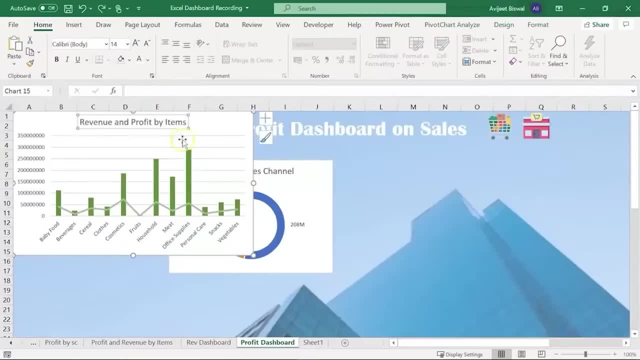 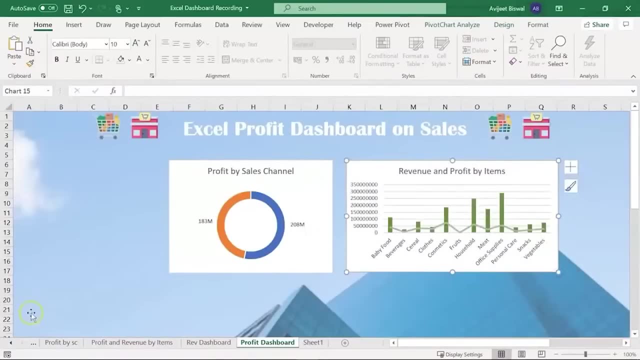 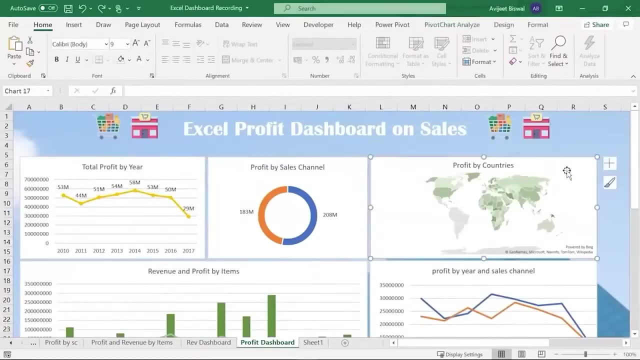 copy this as well. similarly, i will bring the other three charts on to my sales dashboard. ok, so here on my profit dashboard, i have added all the charts and i have aligned and reshaped it so that it looks good. i have also made some formatting. for example, i have reduced the size of 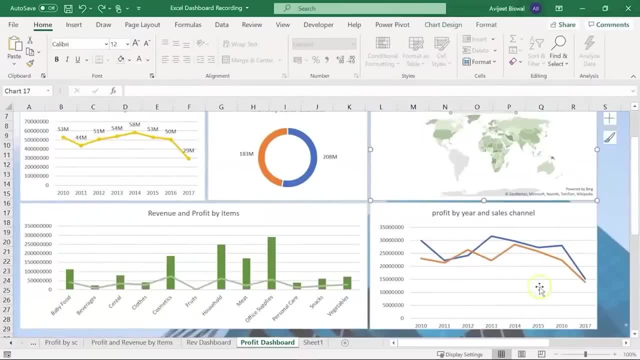 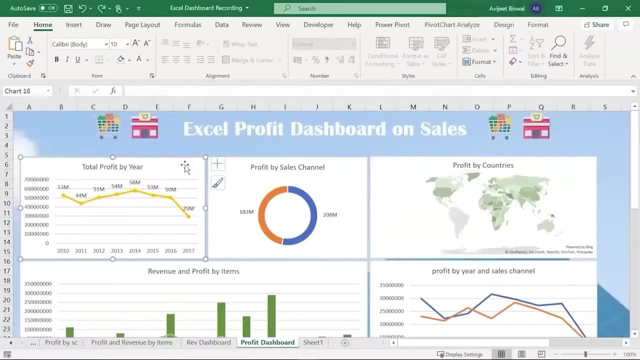 the chart title. now let me go ahead and show you a few more formatting that we also did for the revenue dashboard. first, let's remove the white background from all the charts. so i will select the first chart, i will right click and i will click on format chart. 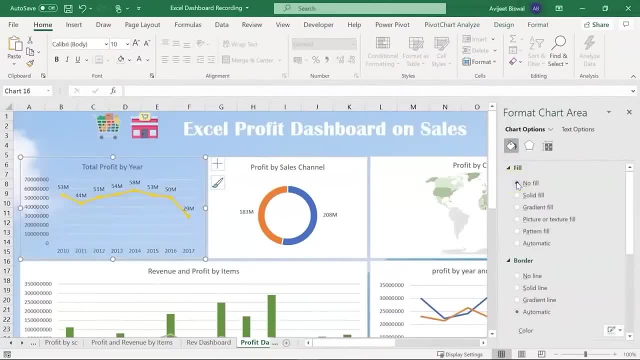 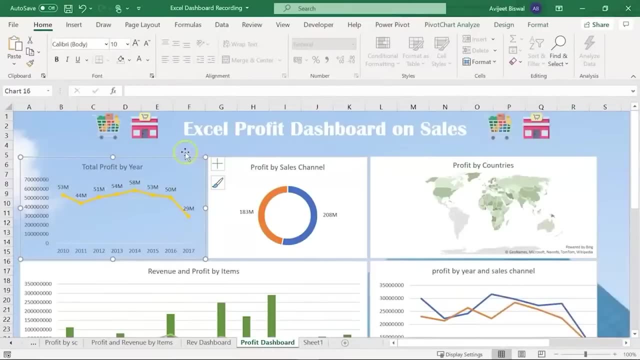 area here under fill, i will select no fill. next, i am going to remove the grid lines, so i will just delete it. let me close this now. we also have a outline, so i will go to design, actually format, and i will remove the outline. next i am going to add: 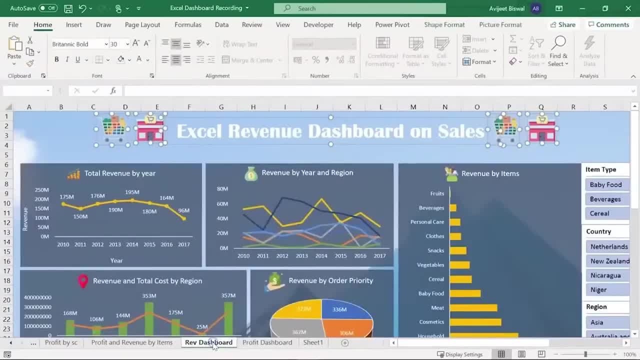 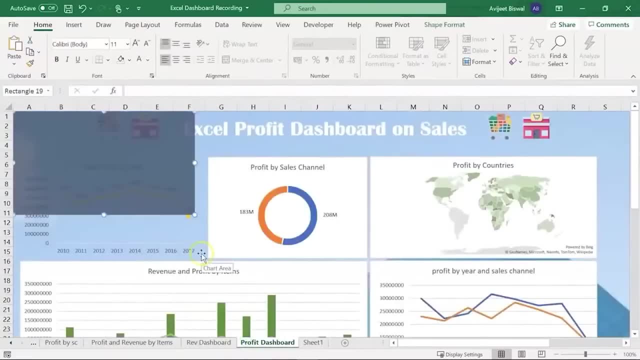 a blue box at the back, like how we did for the revenue dashboard. so let me select a blue box from here and i am going to paste it here. ok, now let me just select the chart and i will bring this to front and i will move this. 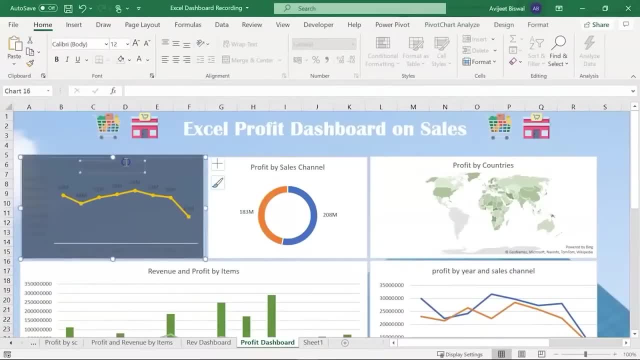 to the back. next, i am going to change the font color all to white, so that it's clearly visible and it's more readable. i will do it for the x axis as well. ok, so here i have my first chart ready. the same i am going to do for the. 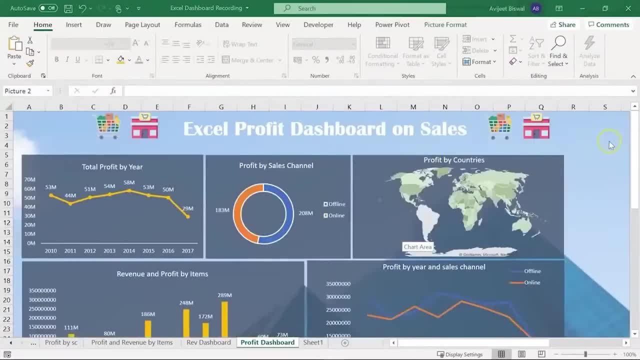 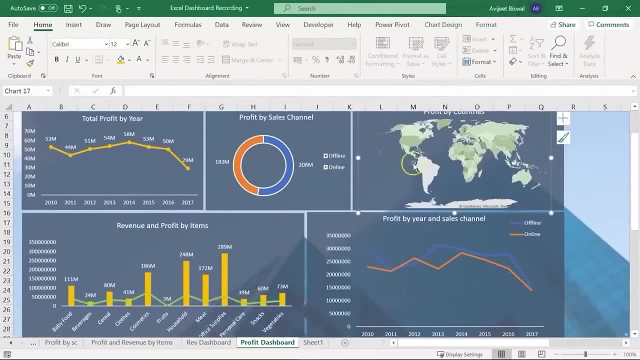 rest of the charts. ok, so now you can see here i have formatted all my charts. i have also added a blue background. you see, here i have also formatted the y labels in terms of millions, which is actually the profit. similarly, here i have added the data labels. 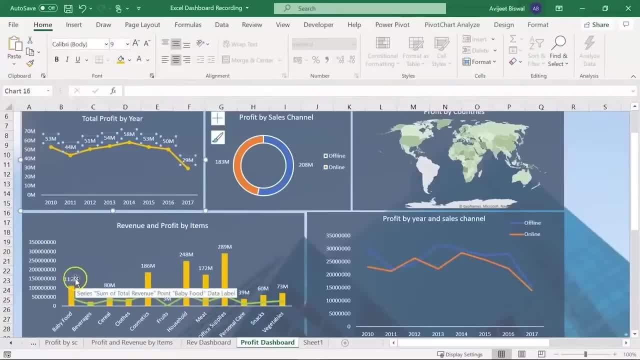 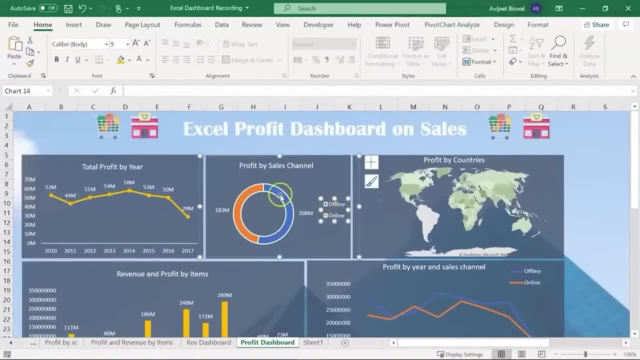 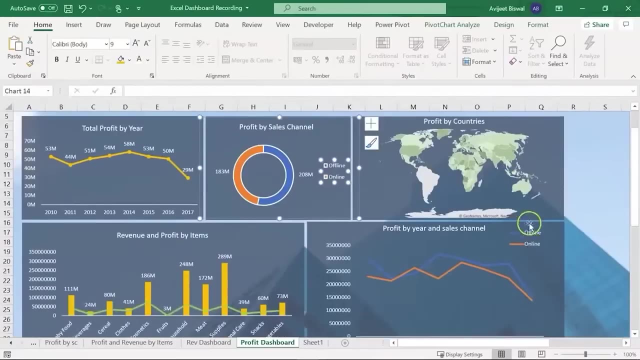 The hiçbir Chart, I'm Going To Format The Chart. Similarly, I'm Going To Format The Chart After Staging My Revenue Return. Then I'm 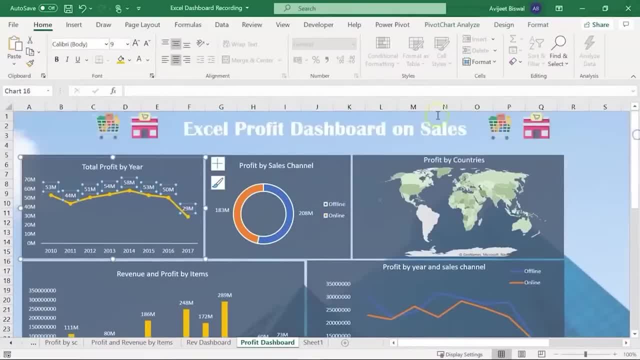 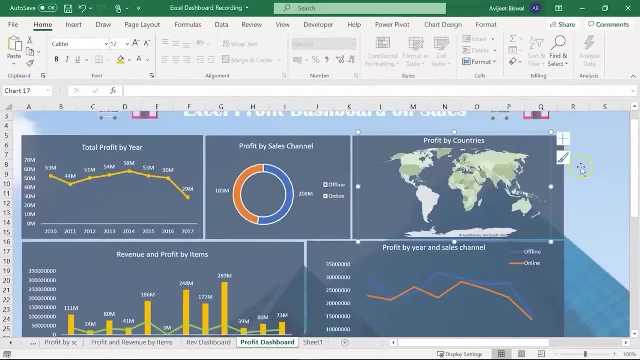 this is for revenue. some of the charts also have the data legend, so here you can see: the blue color represents offline and the red represents online. similarly, here you have the legends. i have also formatted the map as well. ok, now the next thing is to make this. 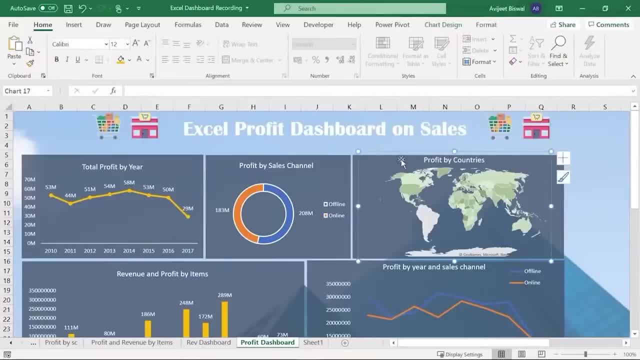 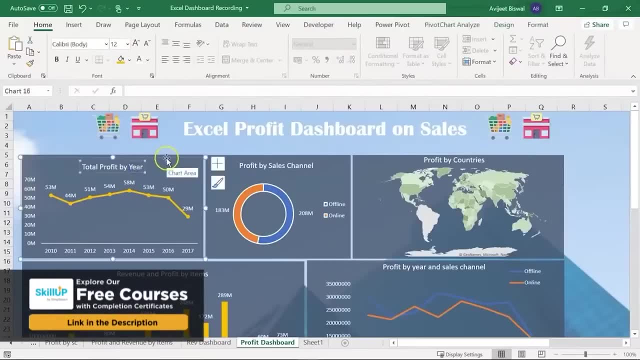 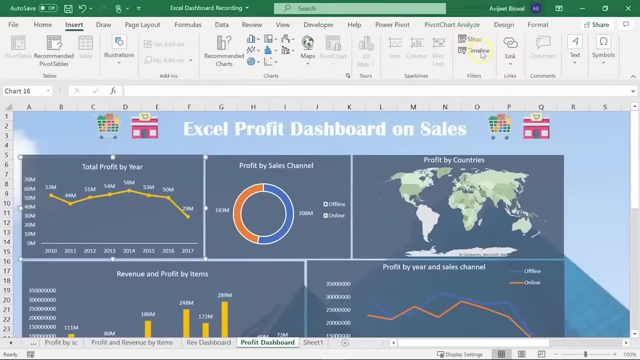 dashboard more interactive, so we will add our slicers as well as timeline. first let me show you how to add a timeline. so i will select one of the charts and i will go to insert. under insert, i have the option to create a timeline, so i will just. 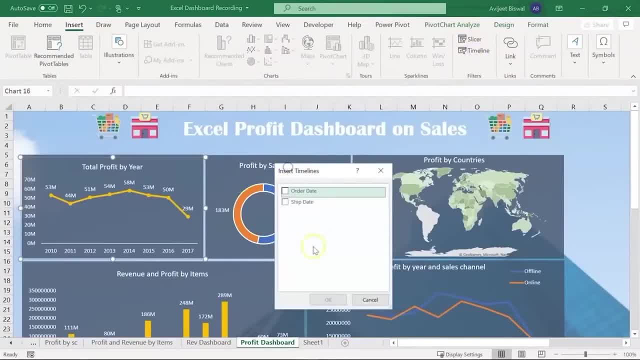 click on timelines, so timeline is actually based on date columns. so since in our data set we only have two date columns- one is order date and one is ship date- so excel has only shown us two columns. so i am going to create my timeline based on order. 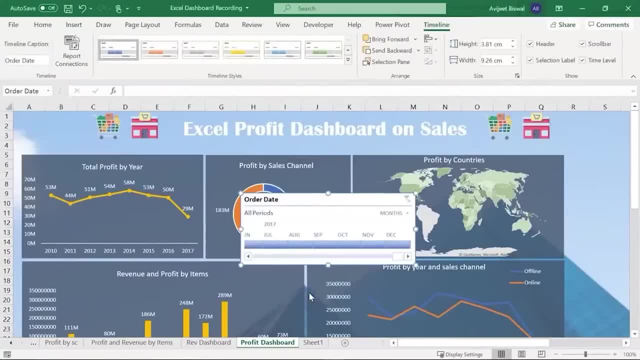 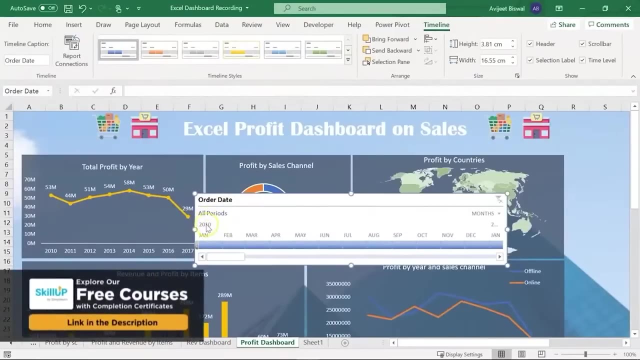 date. so i will select my order date column and i will click on ok. you can see here this is called a timeline. i can expand this now. this timeline is based on months. now if i scroll this timeline, you can see here i have my order year 2010. 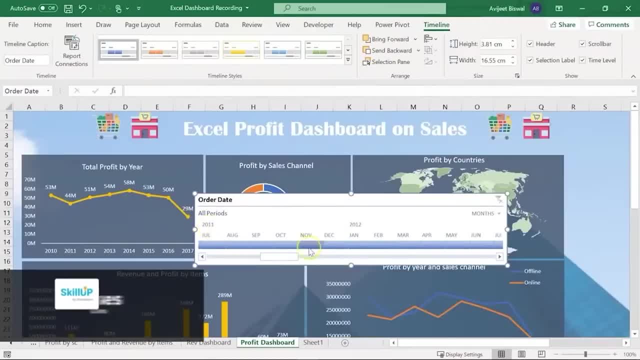 and i have all the 12 months. similarly, we have for 2011, then we have for 2012, all the way till 2017. now you can filter this in terms of years, quarters, months or days. let me just select year now, so i have years. 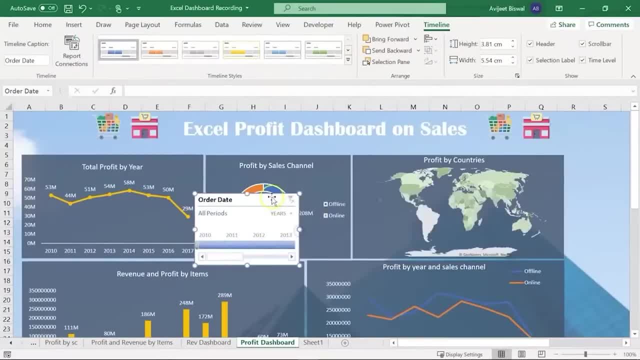 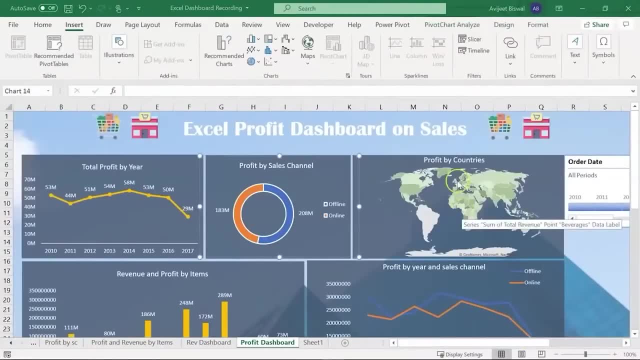 from 2010 till 2017. let me just squeeze this and i will place it somewhere here on the right. now let me go ahead and create a few slicers for my profit dashboard. so i have selected one of the charts under insert. i will click on. 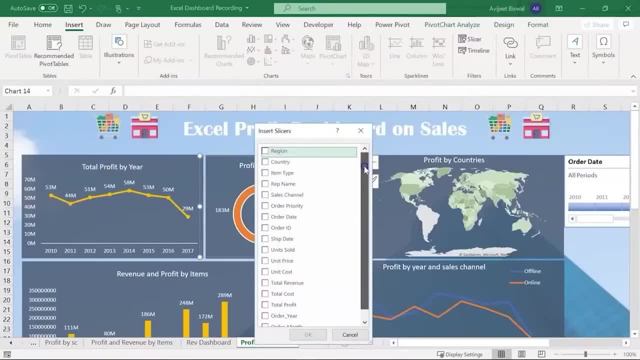 slicer. you can see, it gives me the list of columns from which i want to create slicers, so i will create region. let me also select country. let's say i want the representatives name or the customers name and i will click on ok. so here i have. 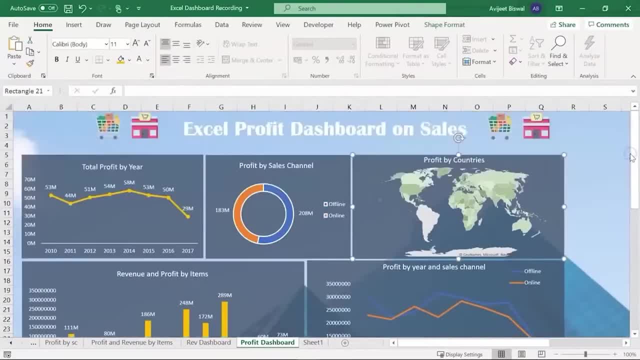 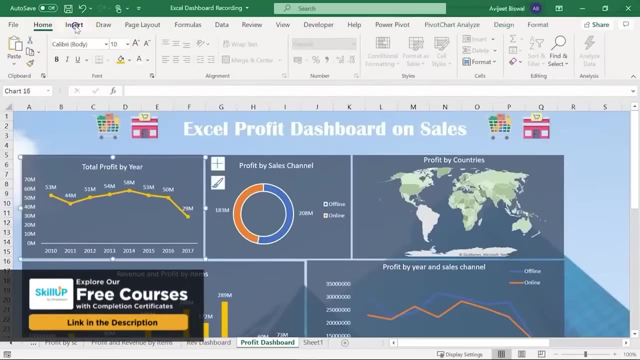 Going To Format In My dashboard more interactive, so we'll add our slicers as well as timeline. first, let me show you how to add a timeline. so I'll select one of the charts and I'll go to insert. under insert, I have the option to create a timeline, so I'll just 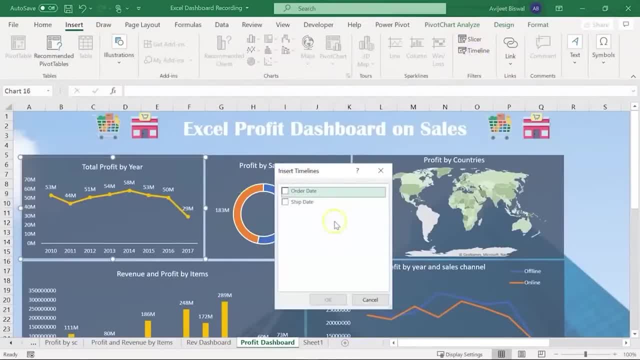 click on timelines, so timeline is actually based on date columns. so since in our data set we only have two date columns- one is order date and one is ship date- so Excel has only shown us two columns. so I'm going to create my timeline based on order date, so I'll select my order date column and I will 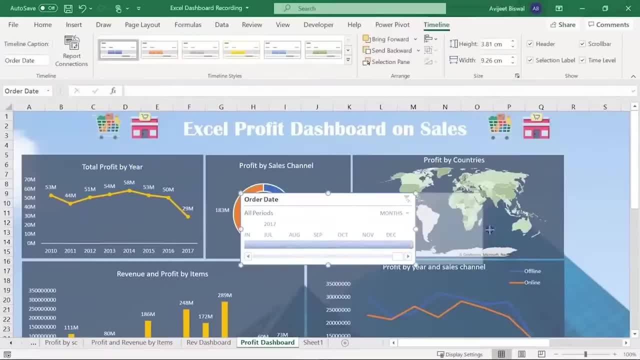 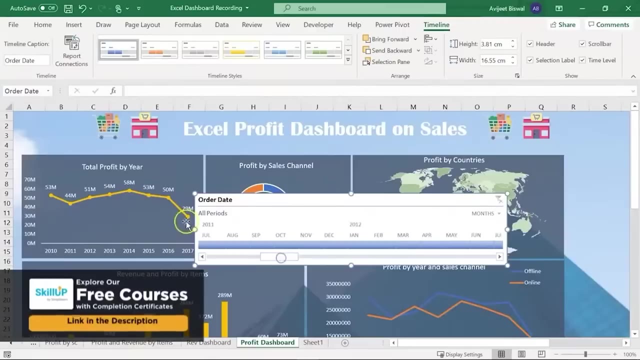 click on OK, you can see here. this is called a timeline. I can expand this now. this timeline is based on months. now, if I scroll this time, you can see here: I have my order year, 2010, and I have all the 12 months. similarly, we have four, 2011, then we have four. 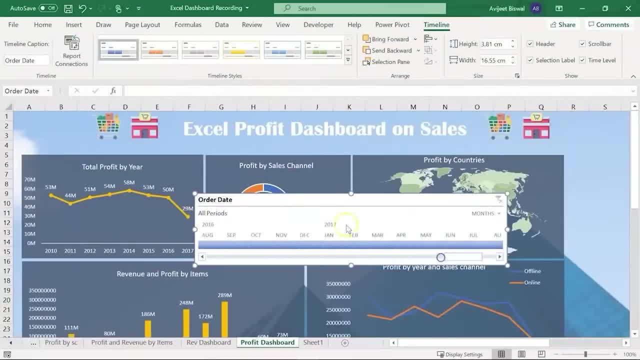 two, three achievement, and then here I have four year year. so if we click on 2012, all the way till 2017- now you can filter this in terms of years, quarters, months or days. let me just select year now, so i have years from 2010 till 2017. let me just 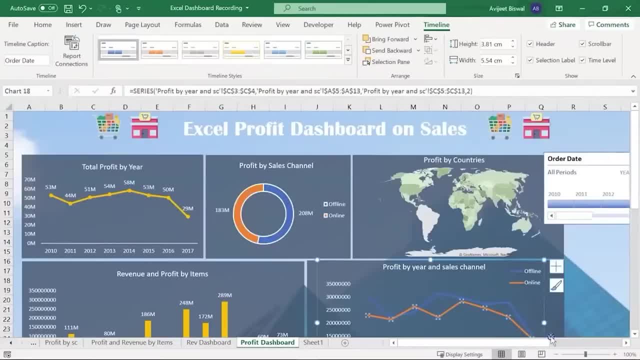 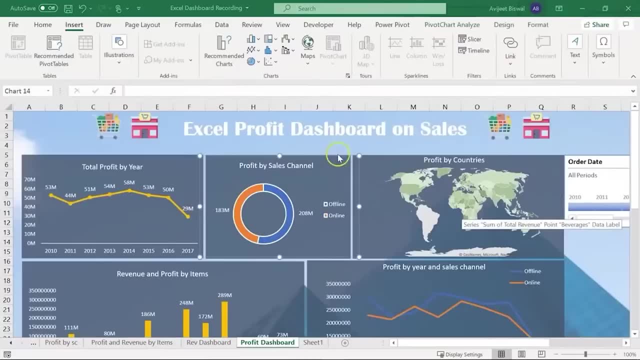 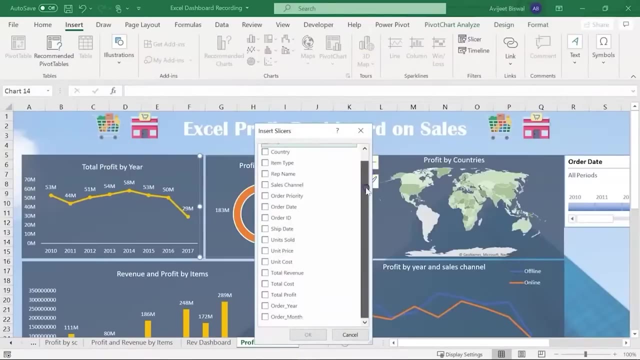 squeeze this and i'll place it somewhere here on the right. now let me go ahead and create a few slicers for my profit dashboard. so i have selected one of the charts under insert. i'll click on slicer. you can see it gives me the list of columns from which i want to create slicers. so i'll create a region. 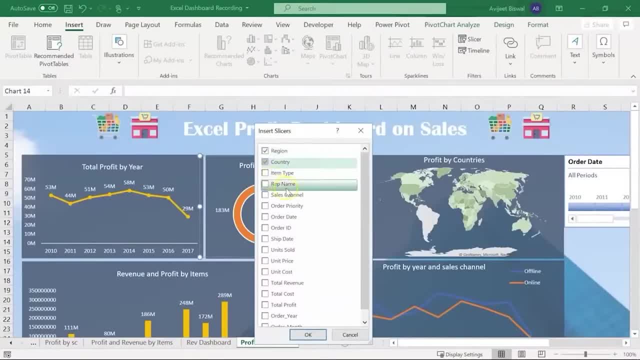 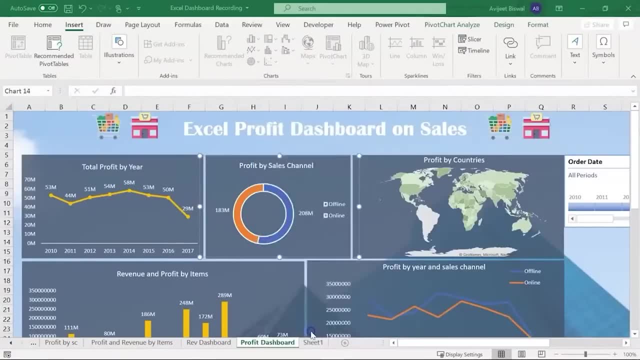 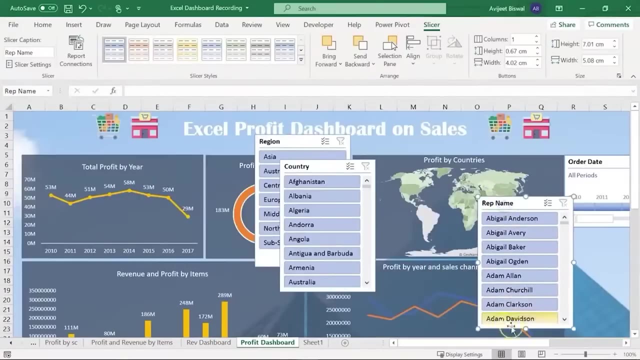 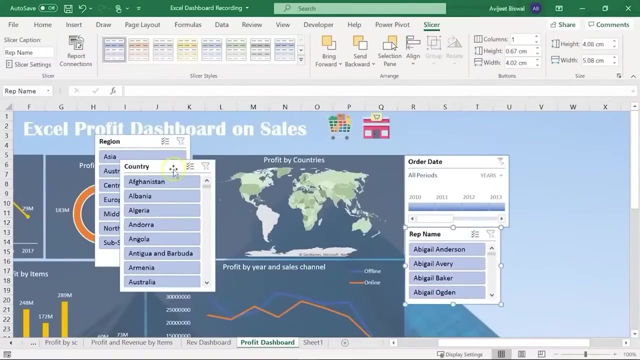 let me also select country. let's say i want the representative's name or the customer's name and i'll click on ok. so here i have created three slicers. let me first resize it and i'll place it on the right. similarly, i'll place the country column also. 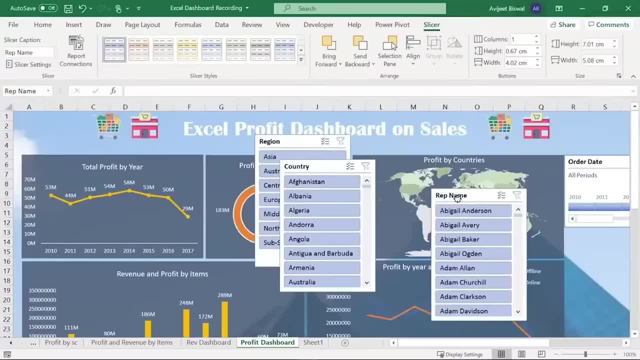 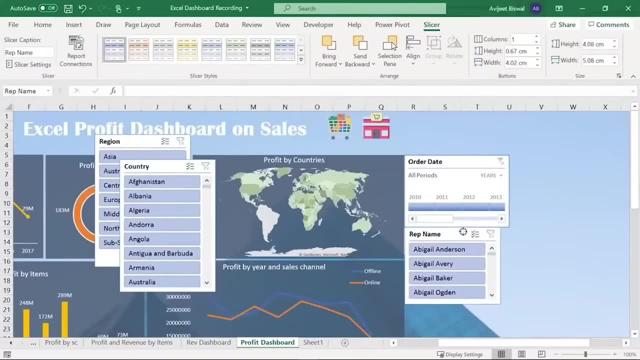 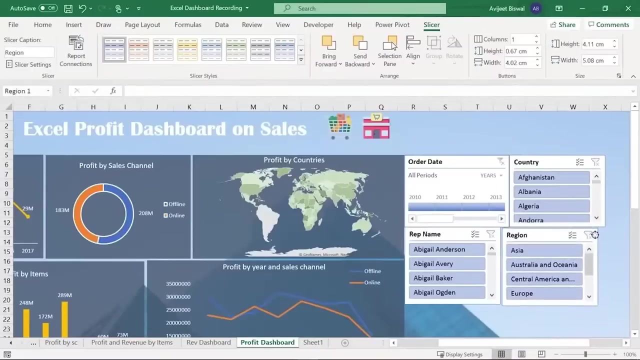 created 3 slicers. let me first resize it and i will place it on the right. similarly, i will place the country column also. then we have the region slicer. i will resize this and i will bring it here. ok, the next thing we need to do is: 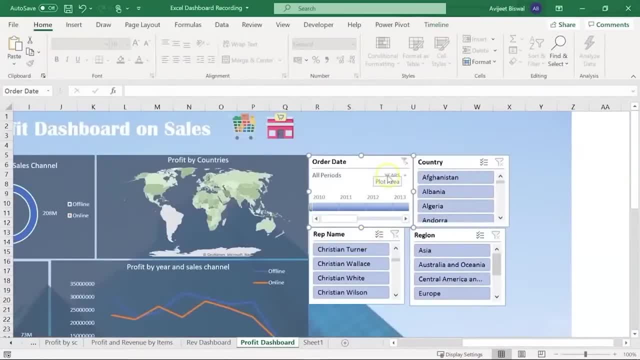 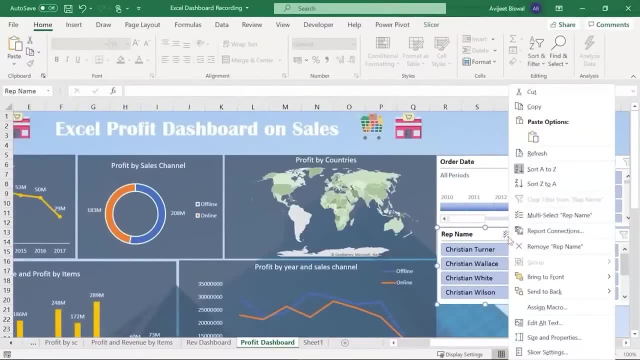 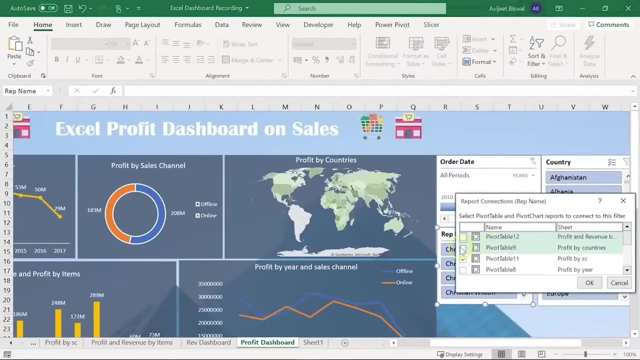 i have to connect all the slicers and the timeline to the pivot tables for the profit dashboard. so i am going to click on the multiple select option and go to report connections. here i am going to select all the pivot tables that are related to profit. so here i have selected. 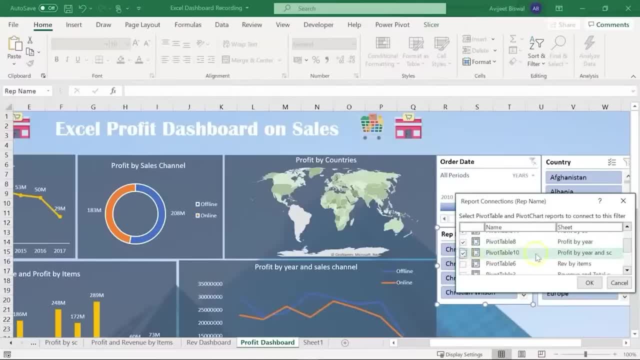 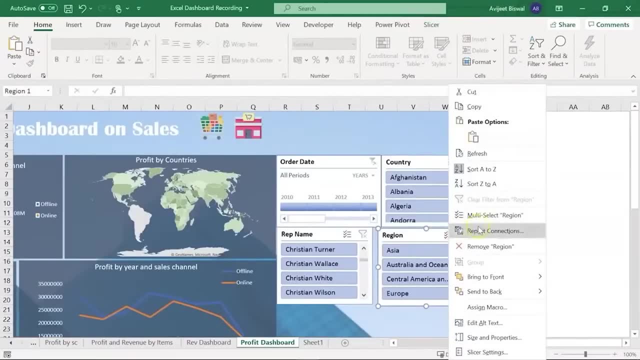 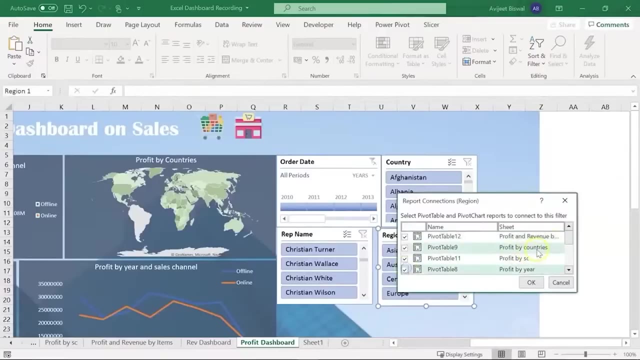 four and i need one more, which is pivot table number 10. i click on ok. similarly, let's create or connect my region filter to all the pivot tables. so i right click go to report connections. here i will choose all my pivot tables which are based on. 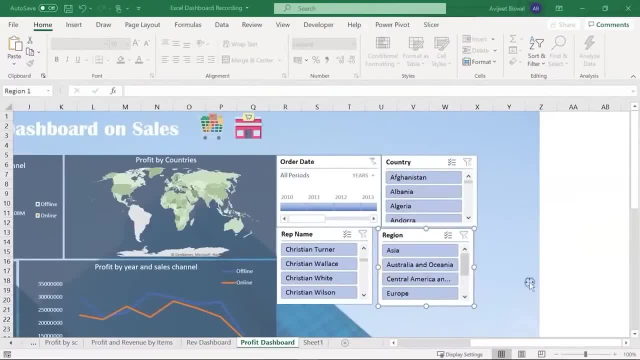 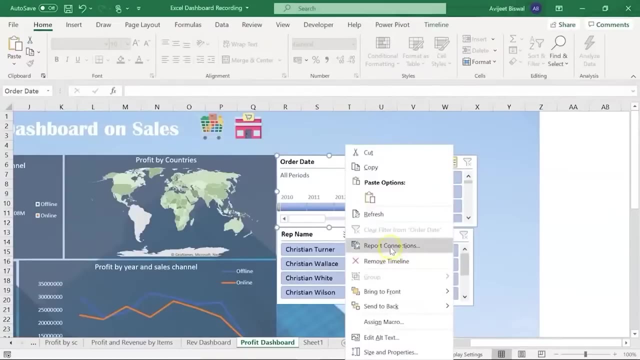 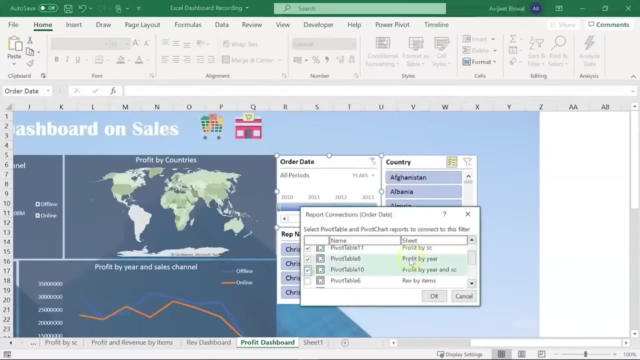 profit, i will click on ok. let's do it for the country slicer as well. click on ok, and similarly i will connect my timeline as well. i will go to report connections and i will select all the pivot tables related to profit. then i will click on ok. 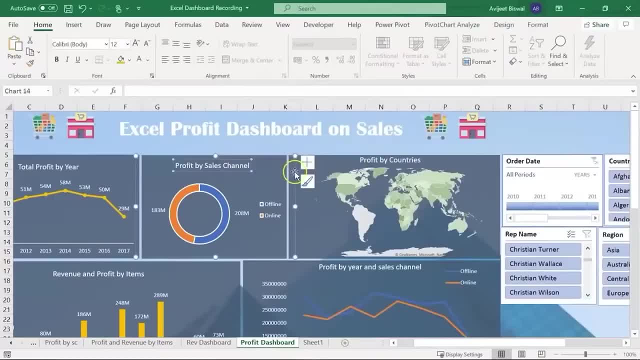 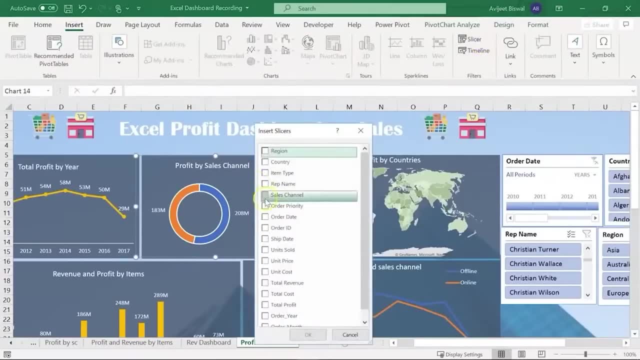 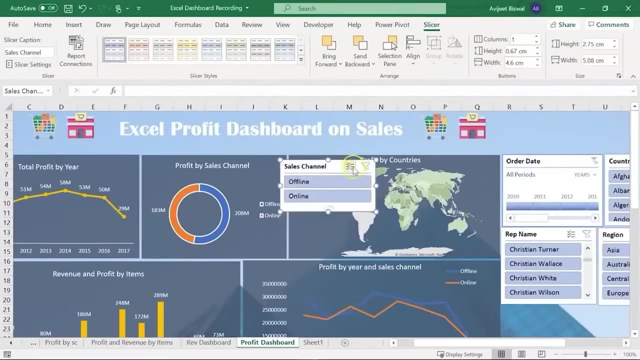 let me now go ahead and create another slicer based on sales channel. so i am selecting one of the pivot charts, i will go to insert, click on slicer and i will select sales channel and hit ok. so i have my sales channel slicer. now let me connect. 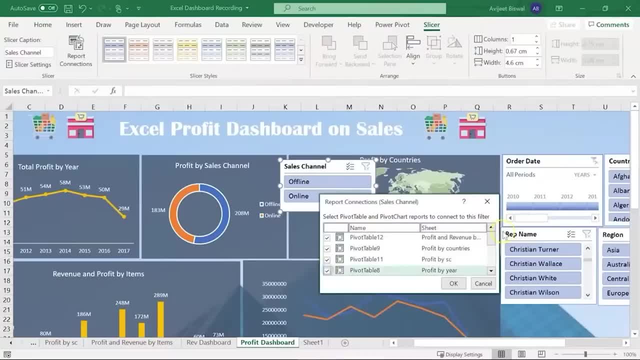 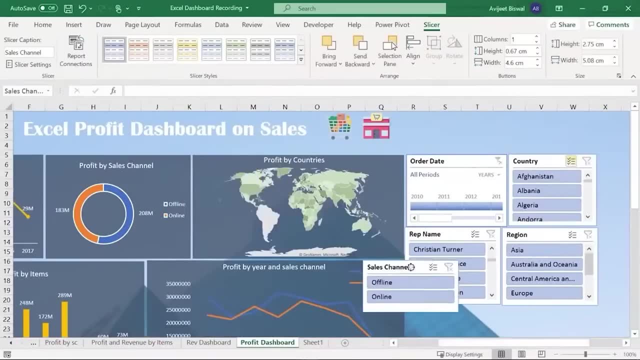 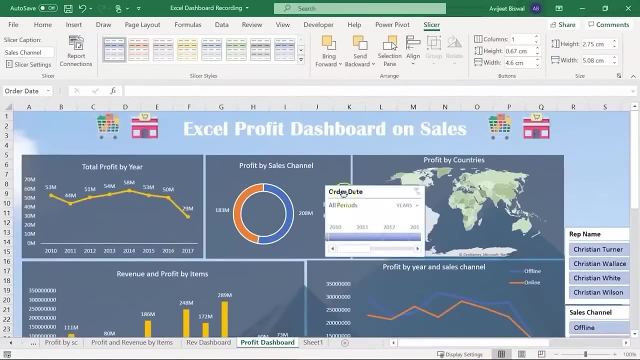 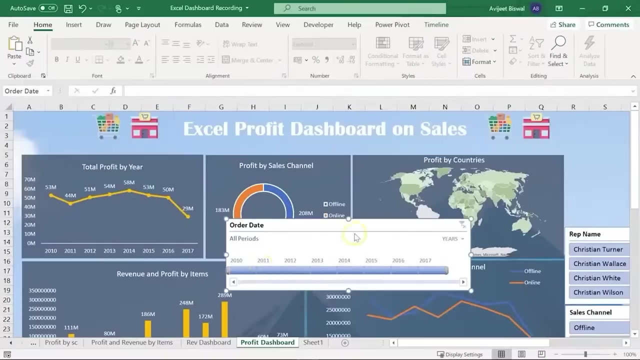 it to all the respective pivot tables that are based on profit. click on. ok, now let me just bring it here. alright, the next thing i want to show is how are we going to use the timeline first. so you see, we have all the years here, from 2010. 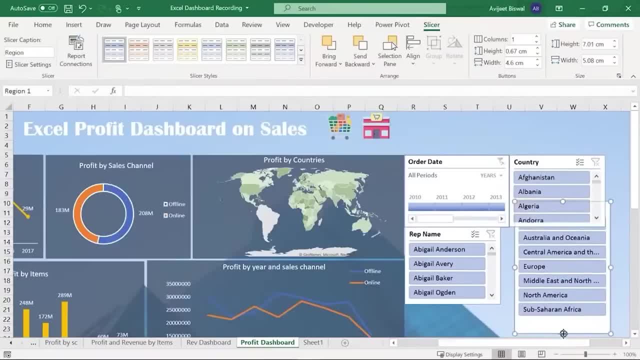 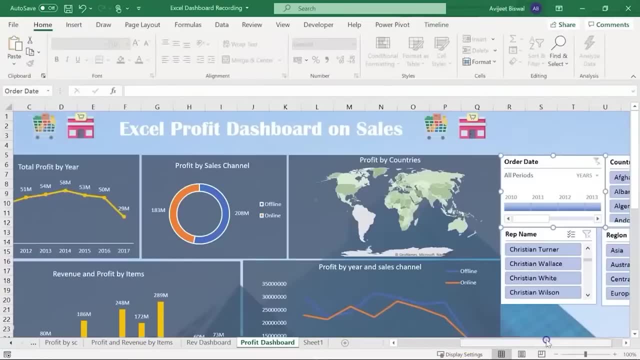 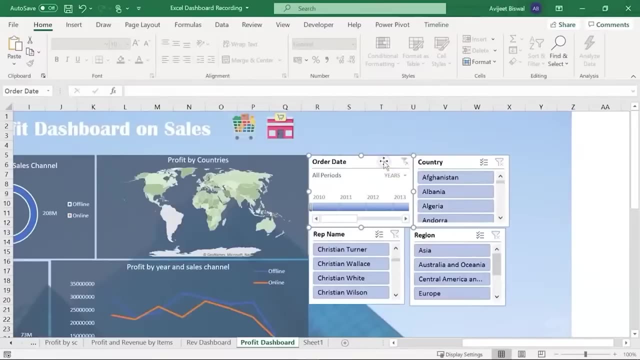 then we have the region slicer. i'll resize this and i'll bring it here. okay, the next thing we need to do is i have to connect all the slicers and the timeline to the pivot tables for the profit dashboard. so i'm going to click on. 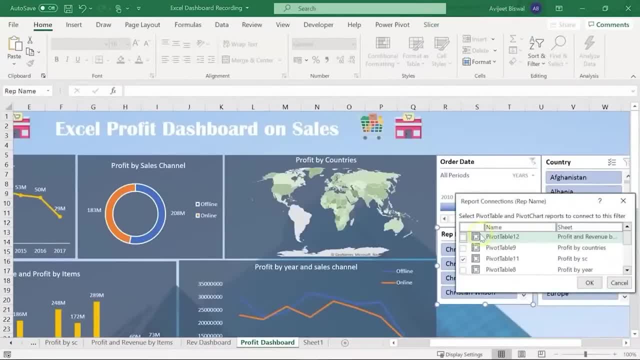 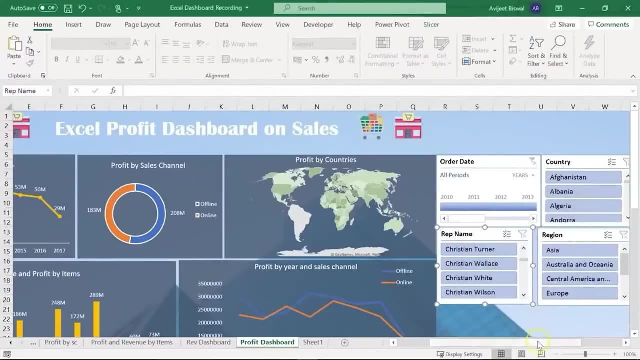 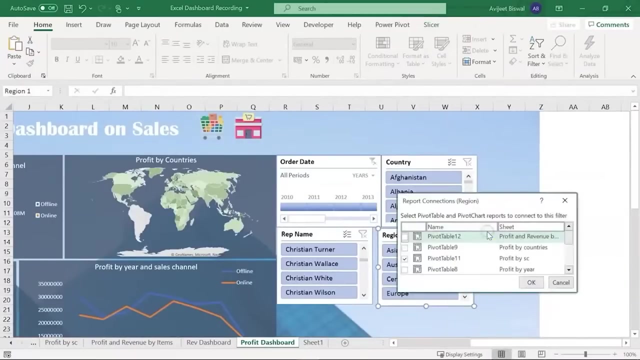 the multiple select option and go to report connections. here i'm going to select all the pivot tables that are related to profit. so here i have selected four and i need one more, which is pivot table number 10. i click on ok. similarly, let's create or connect my region filter to all the pivot tables, so i right click go to report connections. 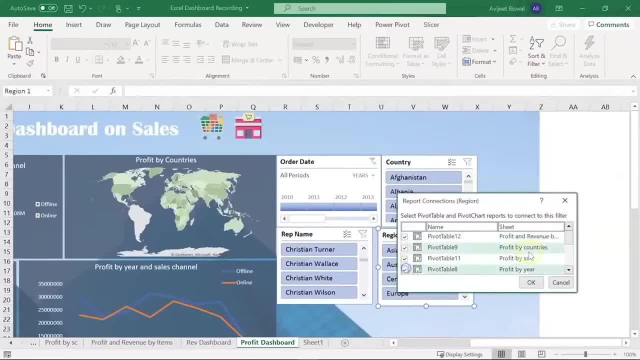 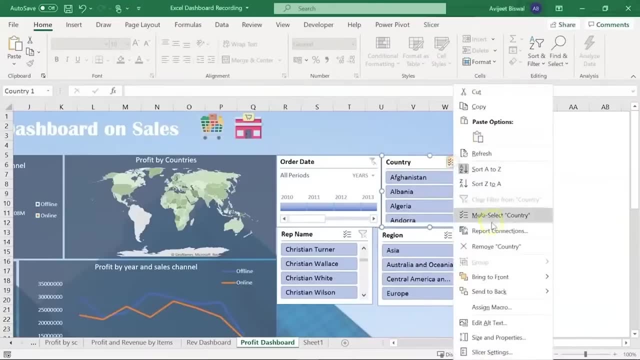 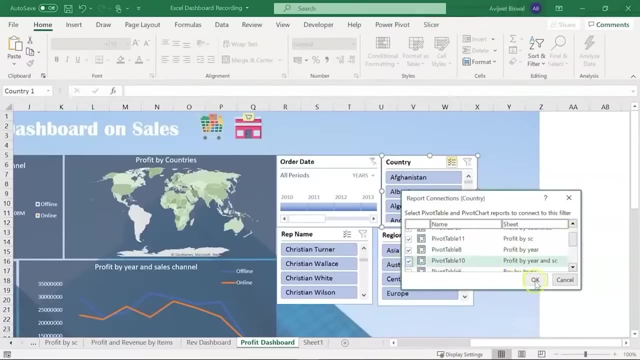 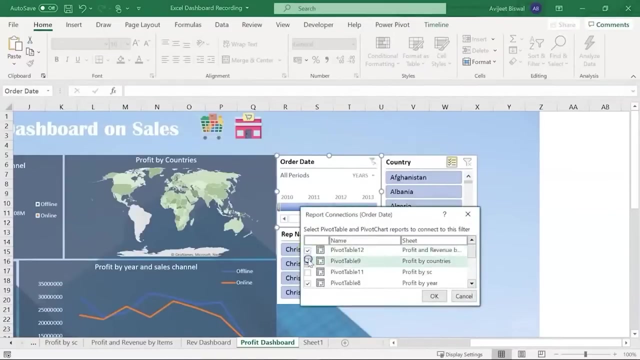 here. i'll choose all my pivot tables which are based on profit. i'll click on ok. let's do it for the country slicer as well. click on ok, and similarly, i'll connect my timeline as well. i'll go to report connections and i'll select. 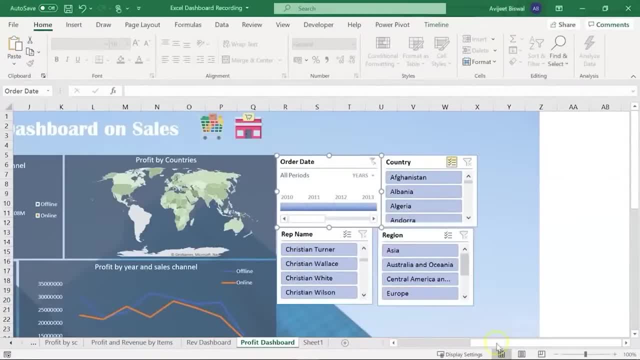 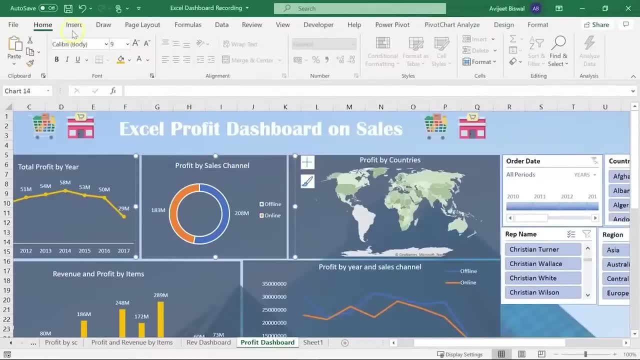 all the pivot tables related to profit, then i'll click on ok. let me now go ahead and create another slicer based on sales channel. so i am selecting one of the pivot charts i'll go to insert, click on slicer and i'll select sales channel and hit ok. 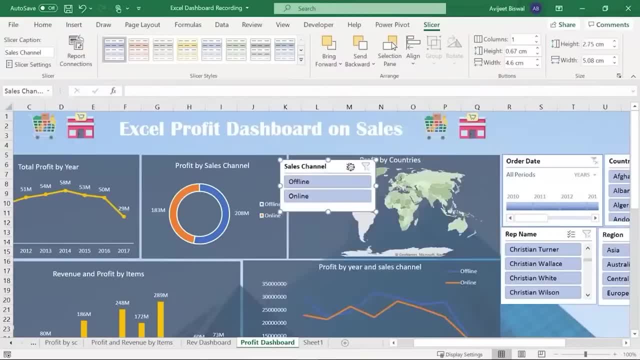 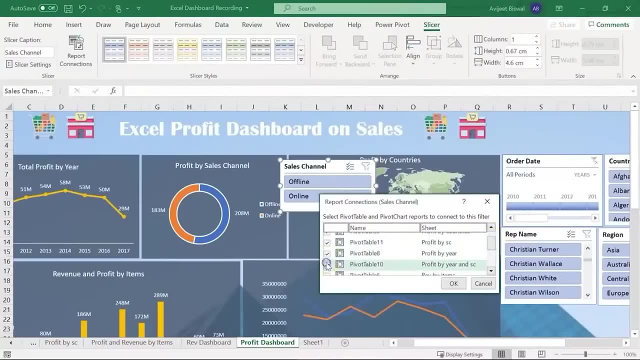 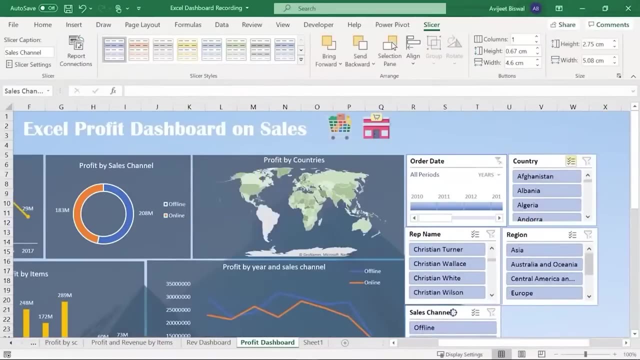 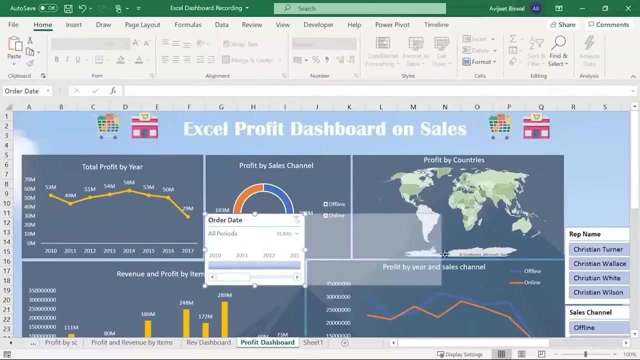 so i have my sales channel slicer. now let me connect it to all the respective pivot tables that are based on profit. click on. ok, now let me just bring it here, all right. the next thing i want to show is how are we going to use the timeline first, 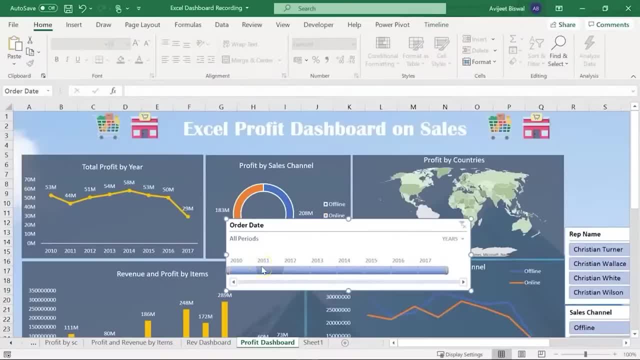 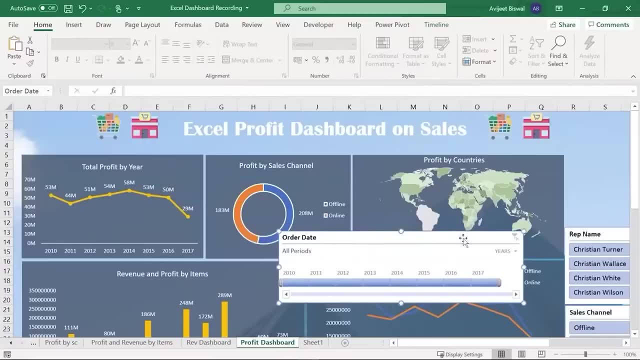 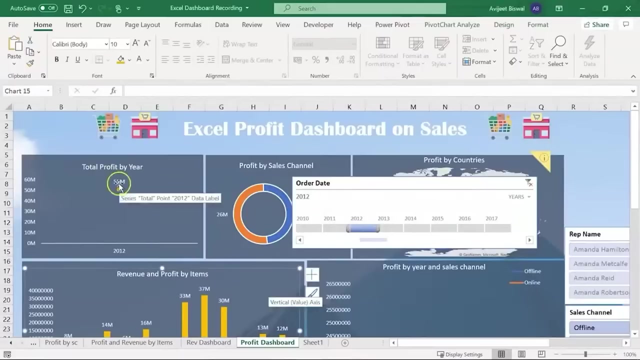 so you see we have all the years here, from 2010 till 2017.. now suppose you want to know the profit that was generated in the year 2012. so i'll just click on this range and now you can see our charts. only so information for 2012. so this dot represents there was 51 million profit. 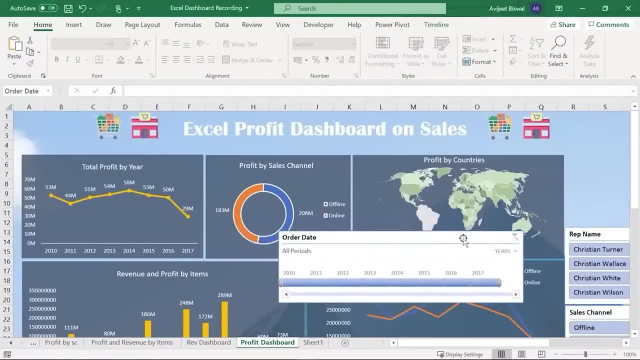 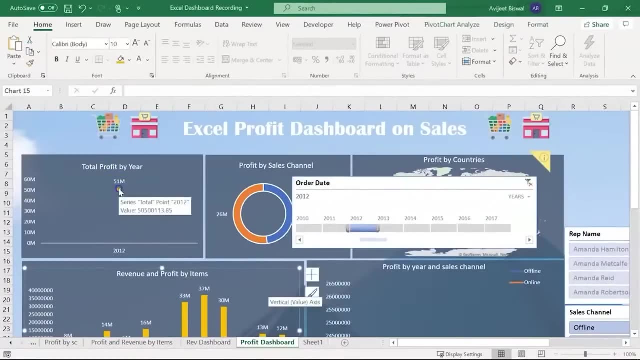 till 2017. now suppose you want to know the profit that was generated in the year 2012, so i will just click on this range and now you can see our charts only show information for 2012, so this dot represents that was 51 million. 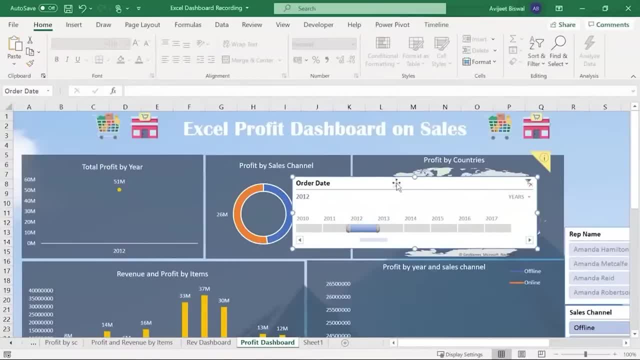 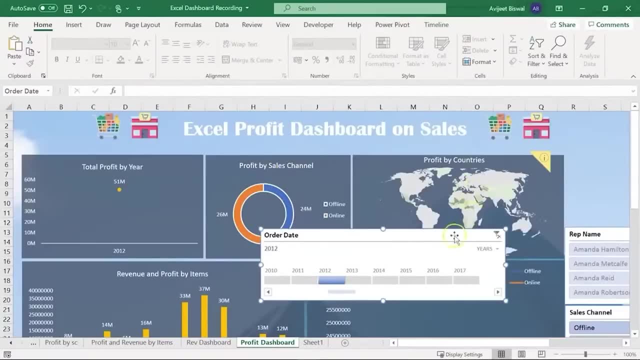 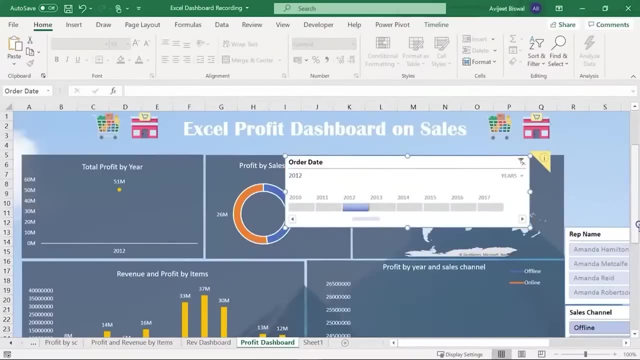 profit in the year 2012. similarly, you can see here the profit by sales channel for 2012. from the map you can see the different countries and the profit each of these countries made in 2012. if i scroll down, you can see the revenue and profit by items. 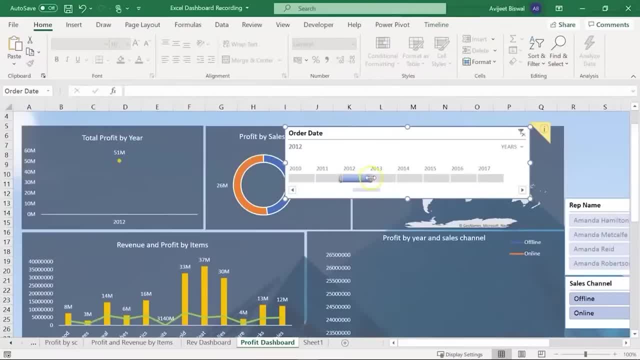 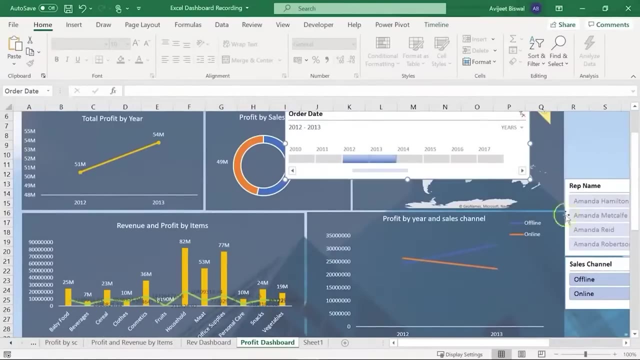 now, if i select another year, lets say 2013, i can just drag this to the right and now you can see our profit by year and sales channel for offline and online. you can see the map or the line chart for total profit by year. so in 2012, 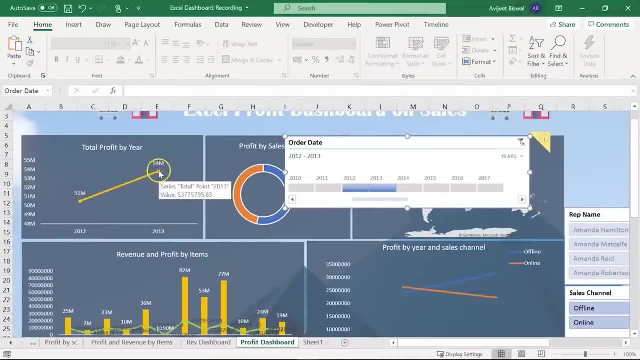 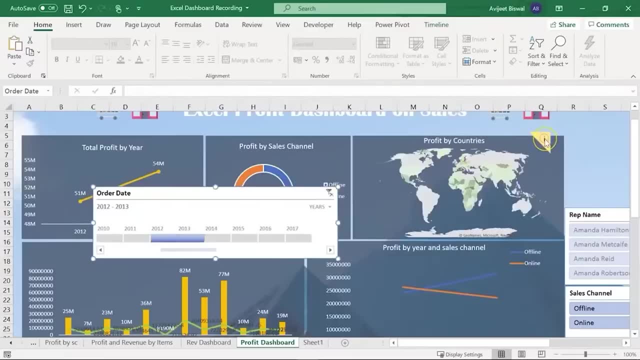 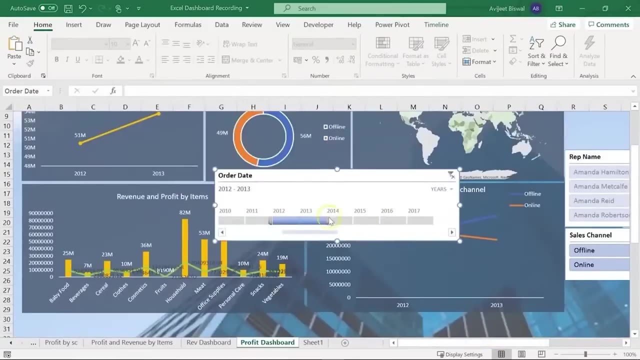 it was 51 million and then it went up to 54 million in 2013. similarly, our map has also changed. now this is sort of an information that we have. you can click on this and check the information that excel has prompted. alright, so this is how you. 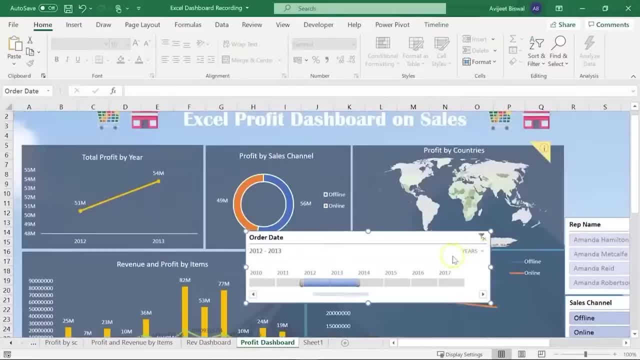 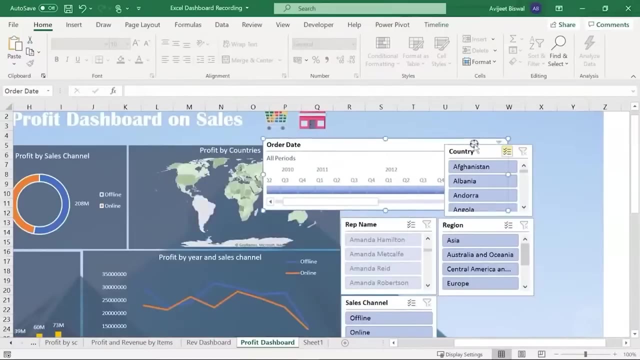 can use a timeline now. as i said, we checked by years. you can also see it for months and quarters as well. let me just uncheck it. i will send it back to the place where it was and i will reduce the size. ok, now suppose you want. 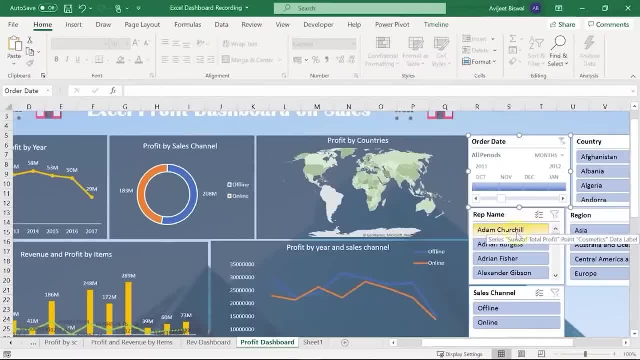 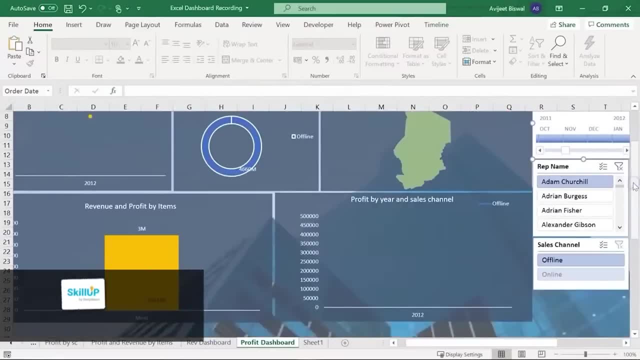 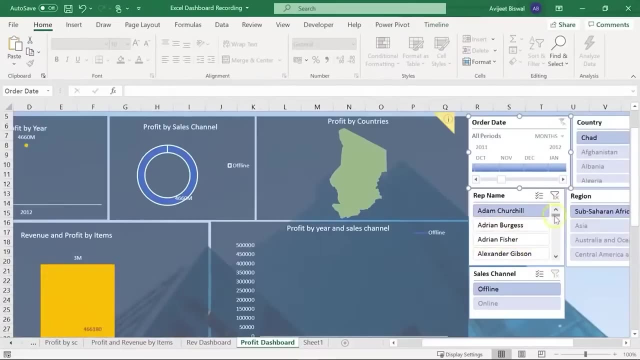 to check the profit made by different representatives. you can select them one by one. let's say Adam Churchill, this is the profit generated by Adam Churchill. similarly, you can select multiple persons as well. now suppose you want to see the profit by different countries, so you can use the 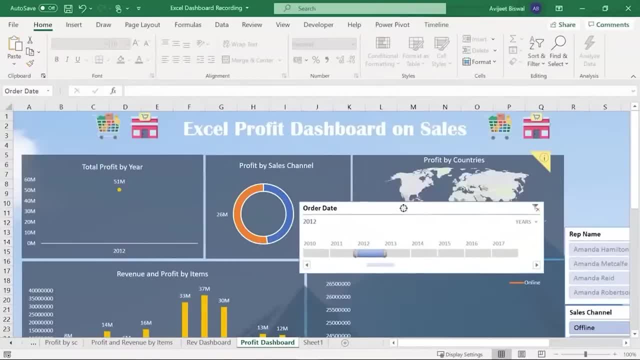 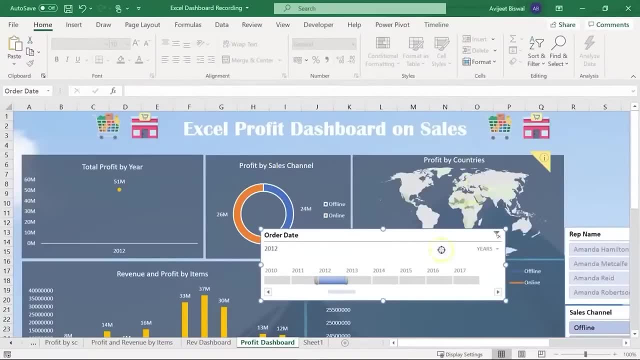 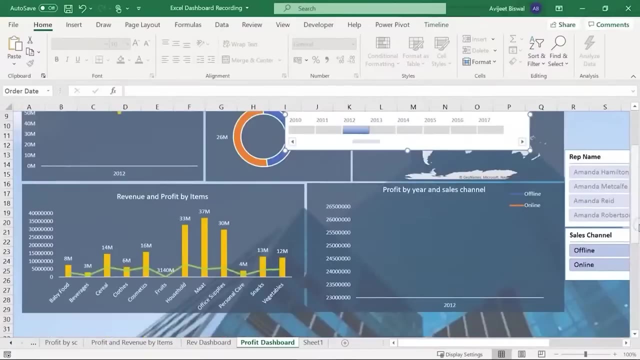 in the year 2012.. similarly, you can see here the profit by sales channel for 2012. from the map, you can see the different countries and the profit each of these countries made in 2012. if i scroll down, you can see the revenue and profit by items. now, if i select, 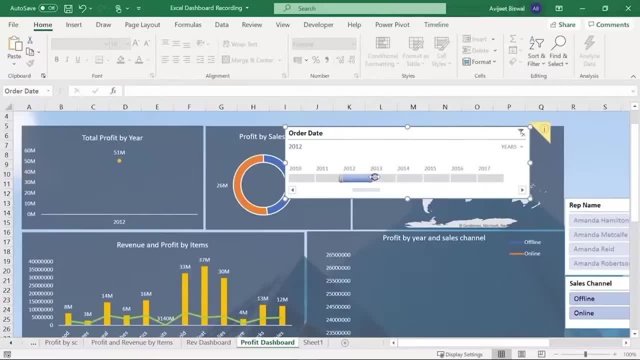 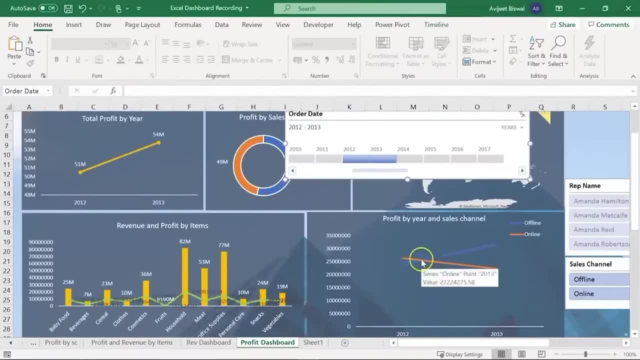 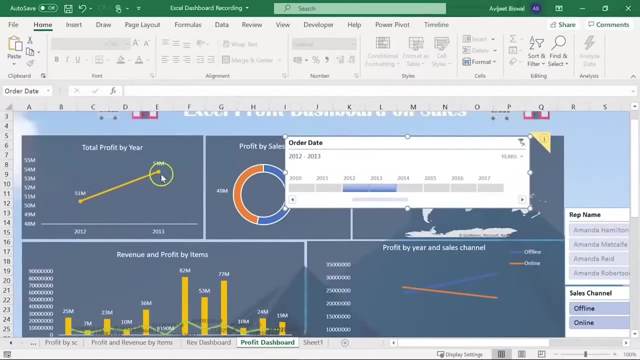 another year, let's say 2013. i can just drag this to the right- and now you can see our profit by year and sales channel for offline and online. you can see the map or the line chart for total profit by year. so in 2012, 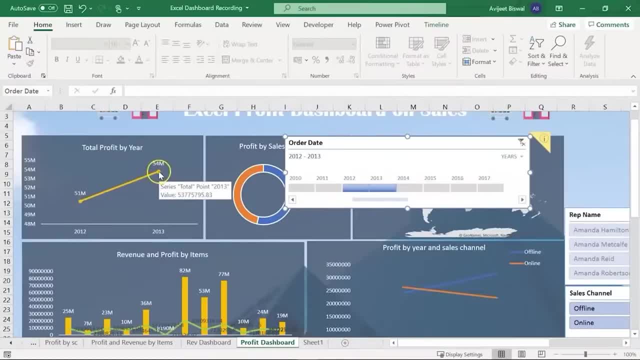 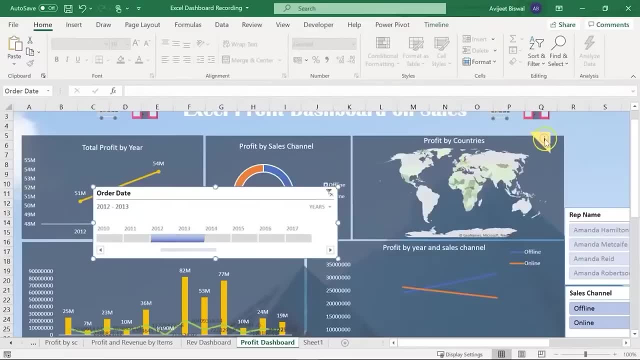 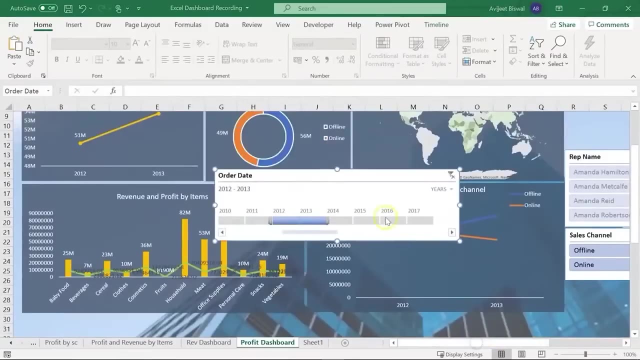 2012 it was 51 million and then it went up to 54 million in 2013.. Similarly, our map has also changed. Now, this is a sort of an information that we have. You can click on this and check the information that Excel has prompted. Alright, so this is how you can use a timeline. 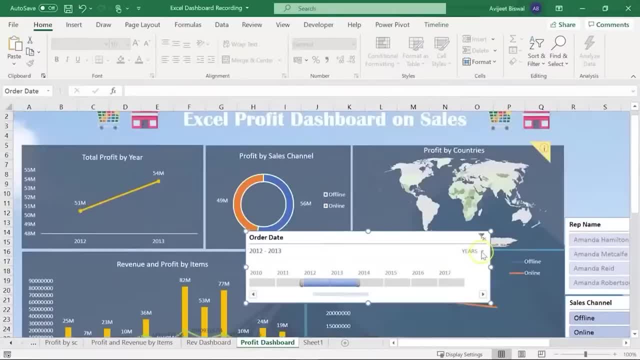 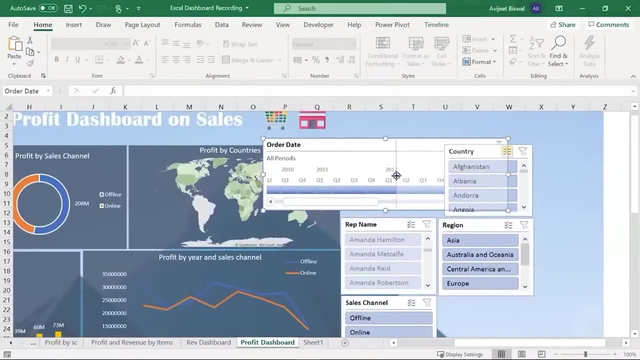 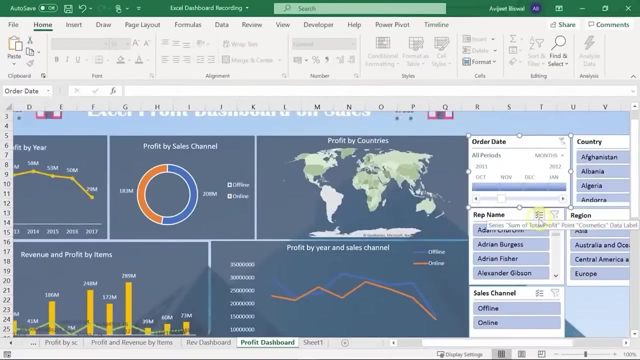 Now, as I said, we checked by years. you can also see it for months and quarters as well. Let me just uncheck it. I'll send it back to the place where it was and I'll reduce the size. Okay, Now suppose you want to check the profit made by different representatives. 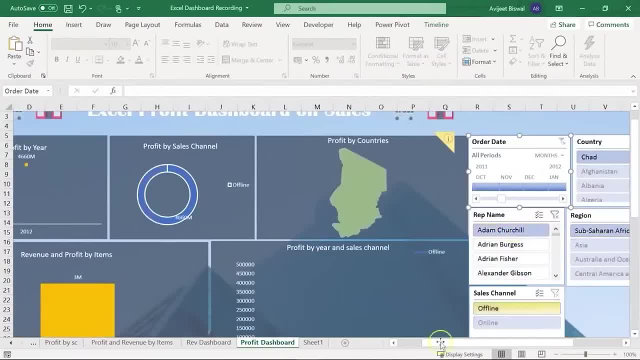 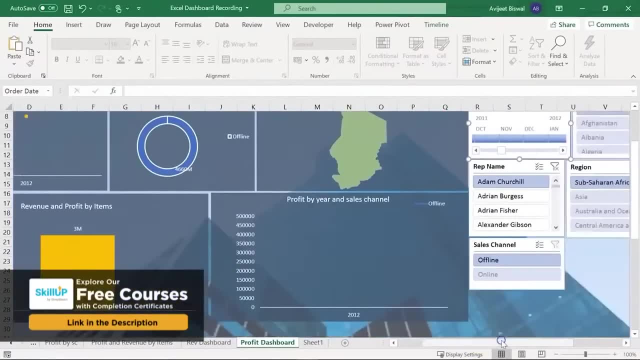 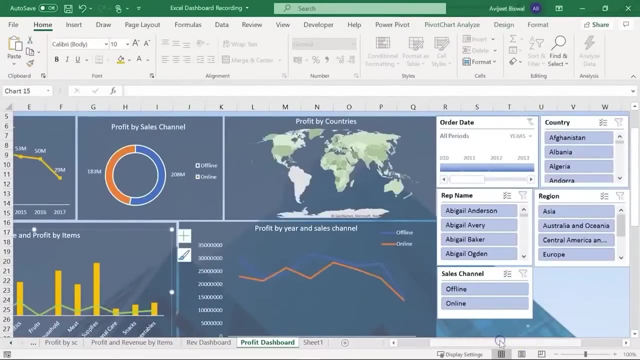 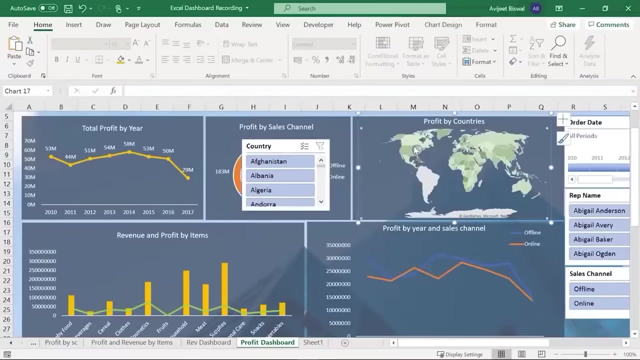 You can select them one by one. Let's say Adam Churchill. This is the profit generated by Adam Churchill. Similarly, you can select multiple persons as well. Now suppose you want to see the profit by different countries, So you can use the country slicer. Let me just bring this to the middle, and let's 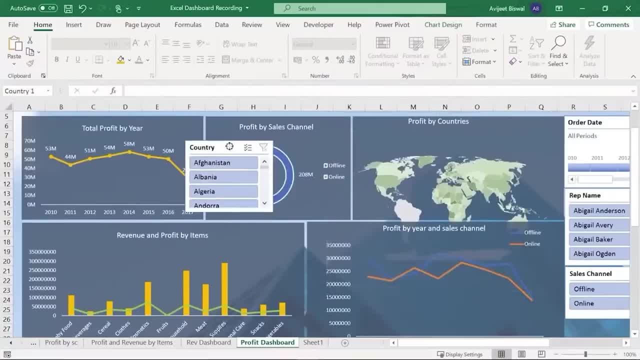 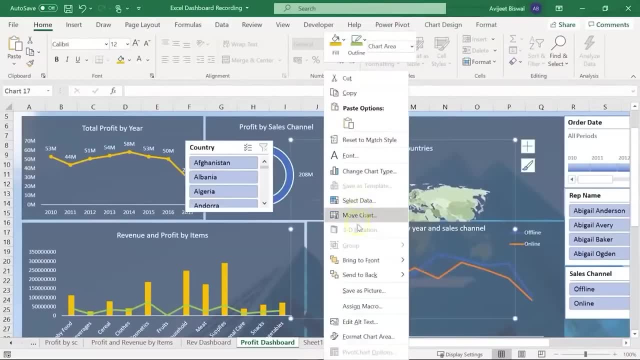 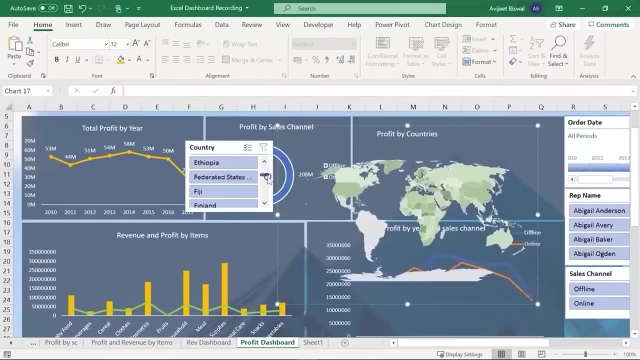 expand our chart a bit. Okay, So here you have the profit by different countries chart. I'll just bring this to the front so that you can see it clearly. Okay, Here, suppose you want to see the profit generated in, let's say, United Kingdom. You can select. 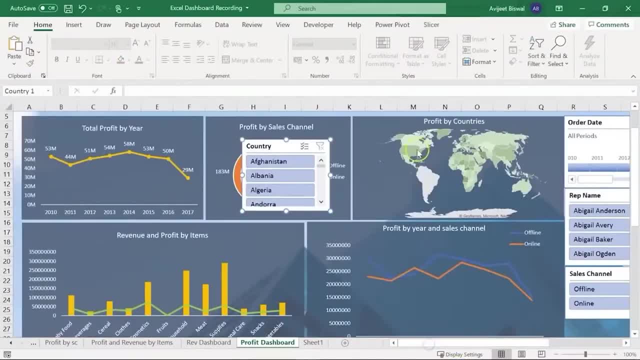 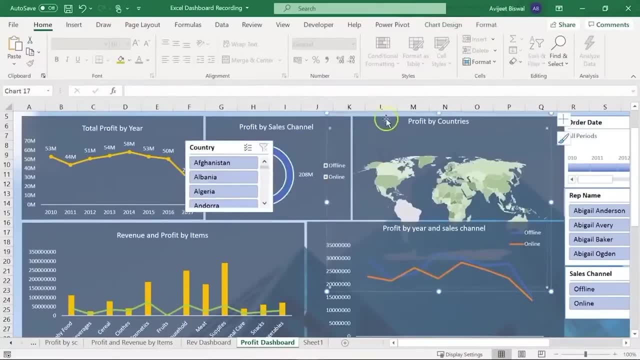 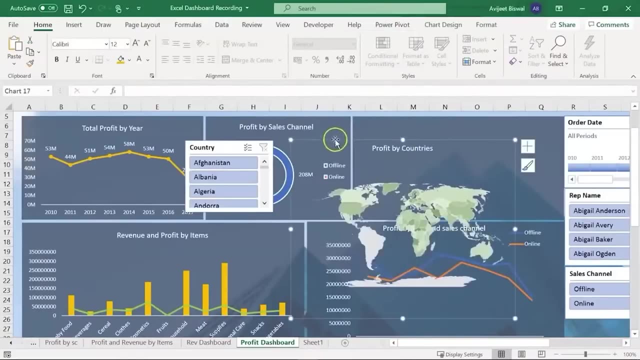 country slicer. let me just bring this to the middle and let's expand our chart a bit. ok, so here you have the profit by different countries chart. i will just bring this to the front so that you can see it clearly. ok, now here. suppose you want to see the 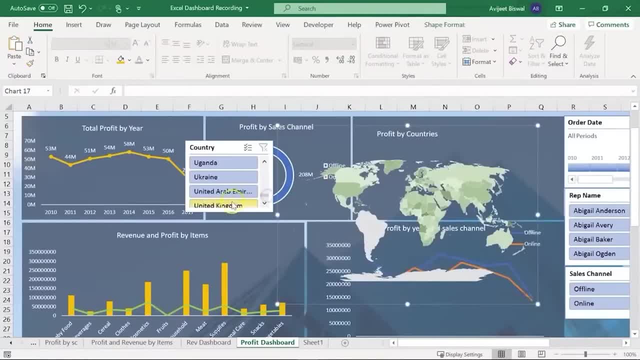 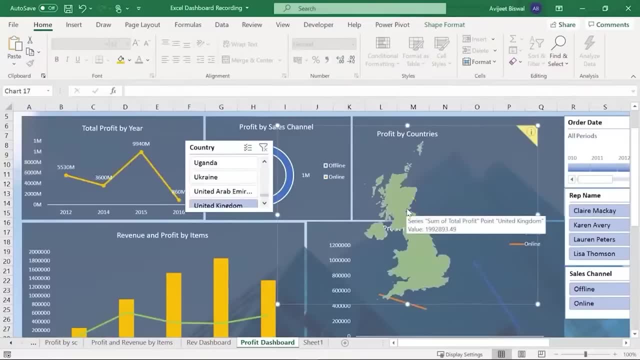 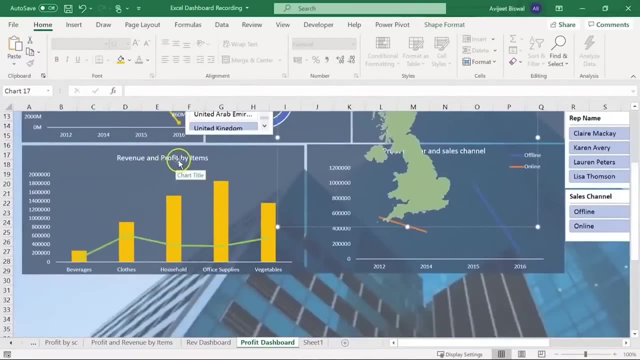 profit generated in, let's say, united kingdom. you can select united kingdom. so this is the map of united kingdom and it tells you the total profit that was generated in united kingdom, and below you can see the revenue and profit for all the items that was sold in. 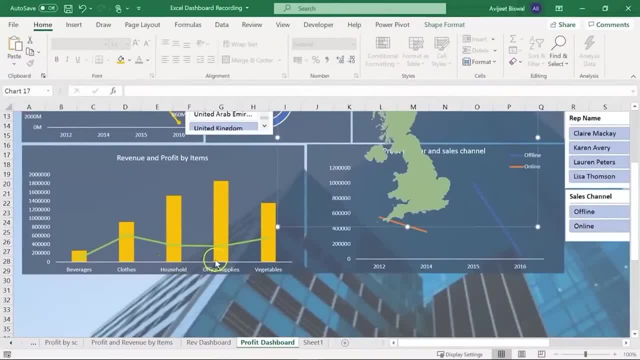 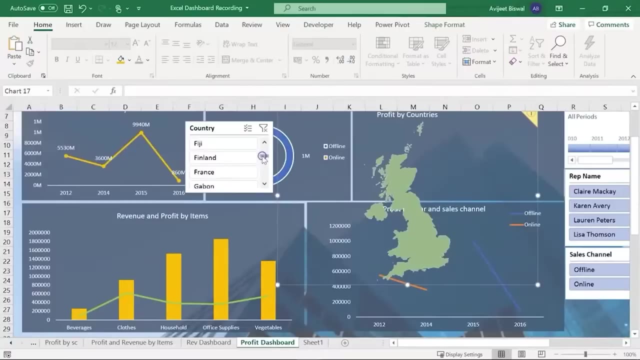 united kingdom. so you had beverages, clothes, household office supplies. so you can see clearly: office supplies item made the highest amount of profit in united kingdom. now you can also select multiple countries. let's say: i want to know for France as well. so my map will change accordingly. 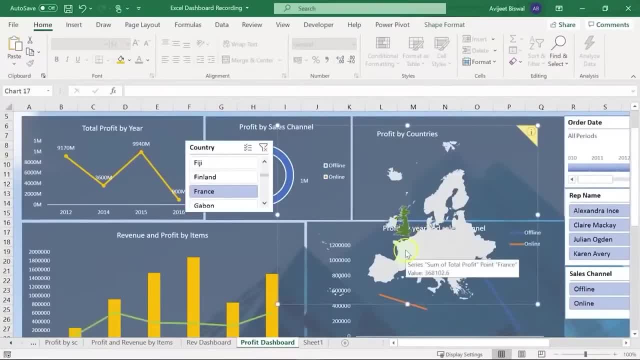 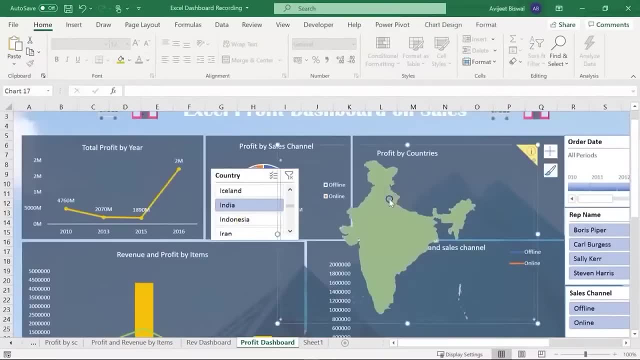 so now i have united kingdom and France selected and the other charts present in my dashboard change accordingly. now i have my country selected as India. you can see the map of India here and these were the respective profit values. now, one thing to note here is: this is actually: 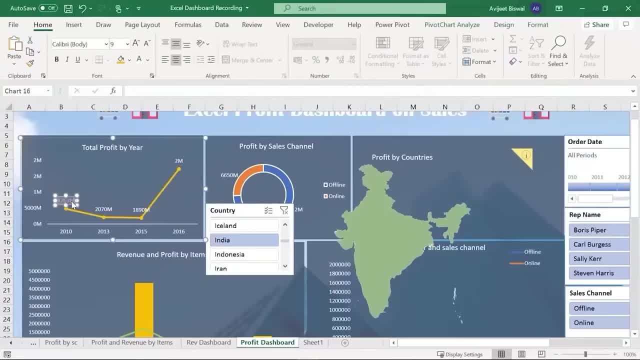 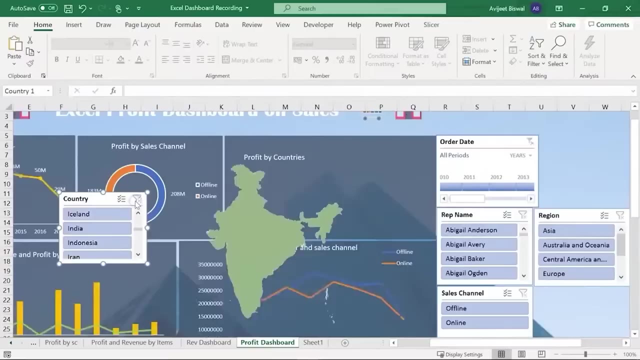 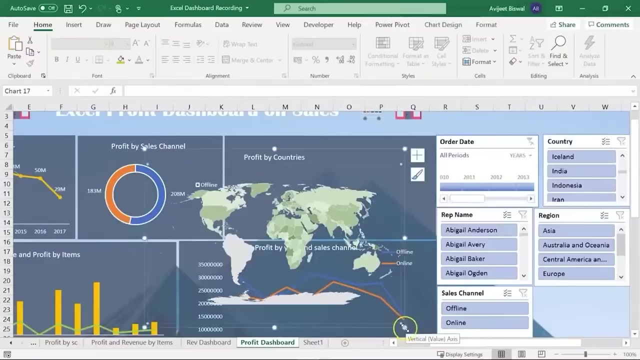 not millions. this should be in K, that is, thousands. so please mark this as thousand and not in millions. even for this, this is actually K and not million. alright, so we have successfully created our second dashboard, that is on profit. let me just resize this a bit and 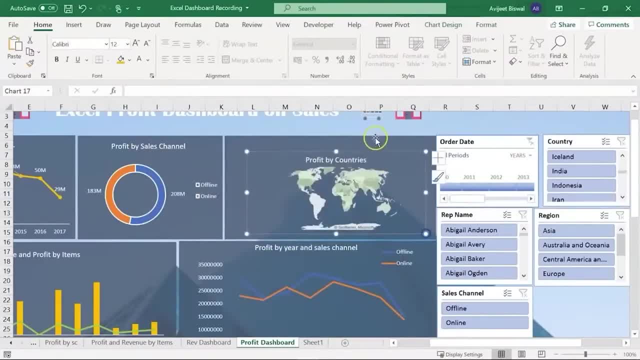 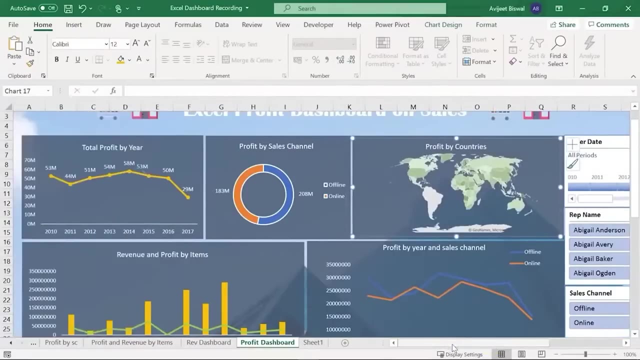 we'll place it where it was earlier. cool. so we saw how to create different pivot tables in pivot charts and then we formatted our pivot charts based on our requirement. we saw how to edit the colors. now let me show you one more thing. you can also change. 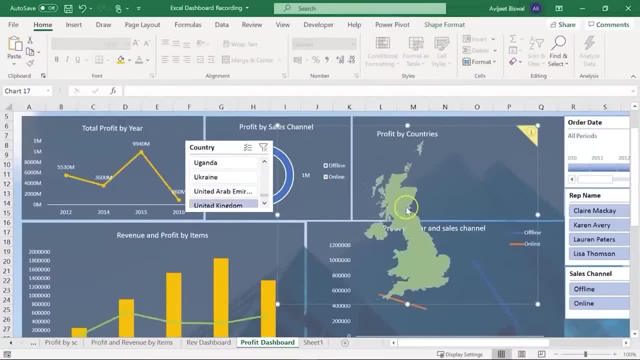 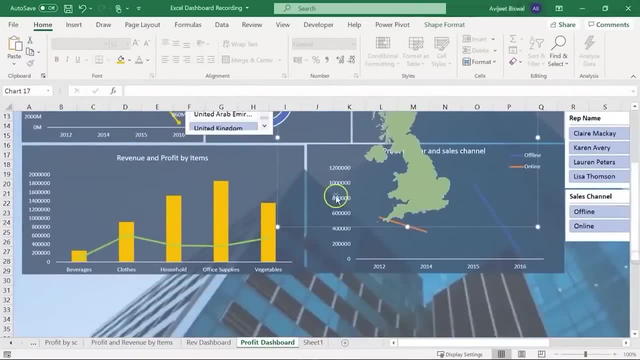 United Kingdom. So this is the map of United Kingdom and it tells you the total profit that was generated in United Kingdom And below you can see the revenue and profit for all the items that was sold in United Kingdom. So you had beverages, clothes, household. 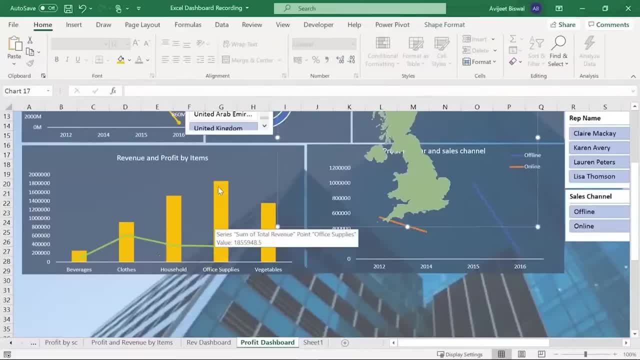 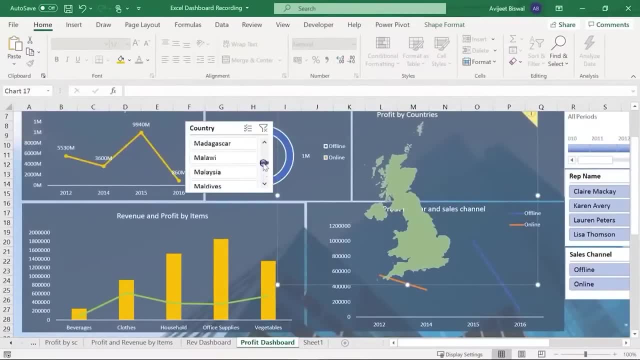 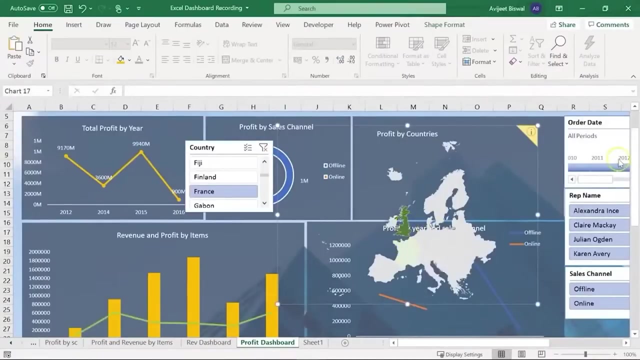 office supplies. so you can see clearly: office supplies item meet the highest amount of profit in united kingdom. now you can also select multiple countries. let's say, i want to know for france as well, so my map will change accordingly. so now i have united kingdom and france selected and 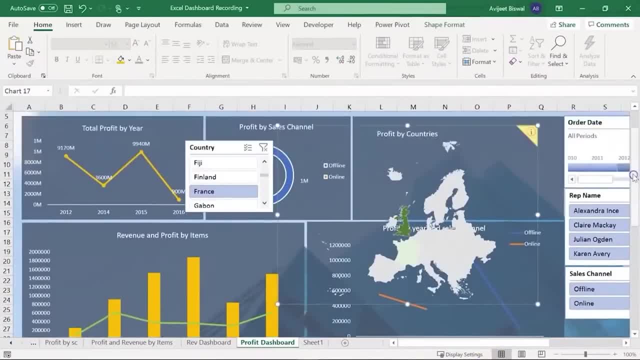 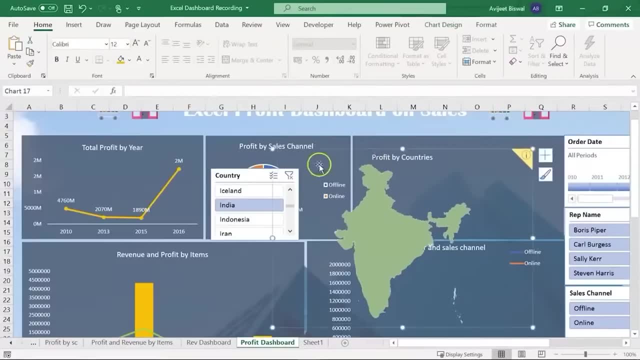 the other charts present in my dashboard change accordingly. now i have my country selected as india, you can see the map of india here and these were the respective profit values. now one thing to note here is: this is actually not millions. that should be in k, that is thousands. so 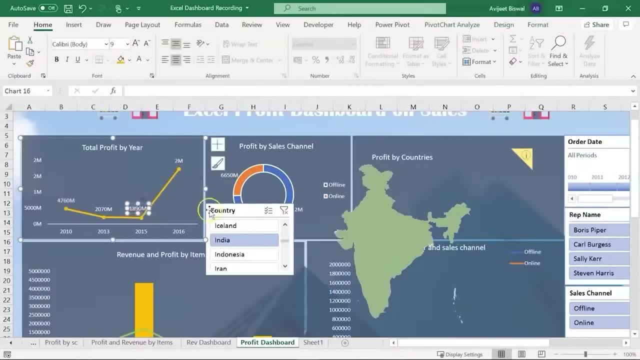 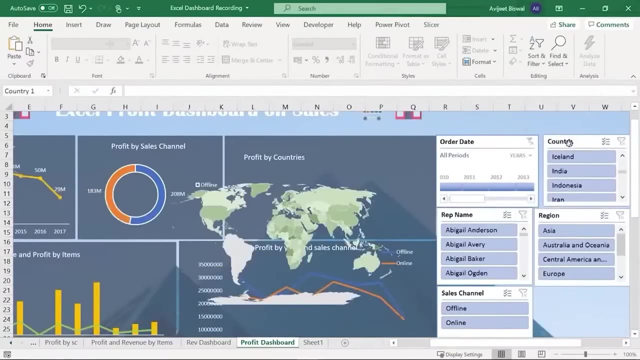 please mark this as thousand and not in millions. even for this, this is actually a k and not million. all right, so we have successfully created our second dashboard that is on profit. let me just resize this a bit and we'll place it where it was earlier. cool. 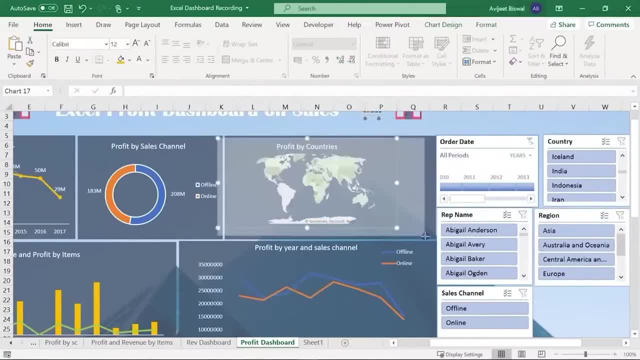 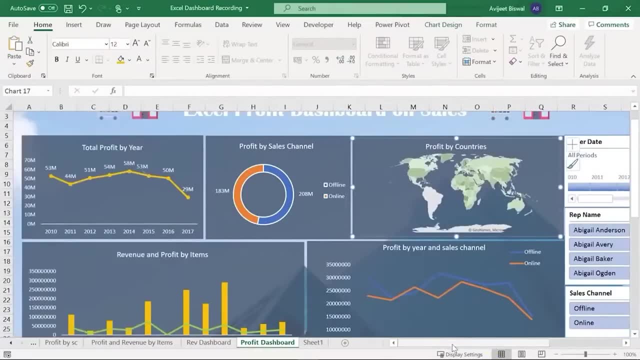 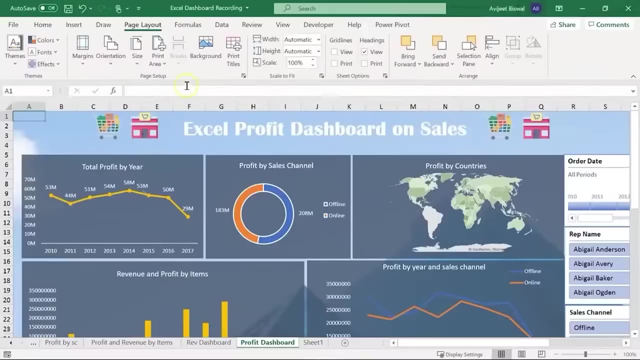 so we saw how to create different pivot tables in pivot charts, and then we formatted our pivot charts based on our requirement. we saw how to edit the colors. now let me show you one more thing. you can also change the look and feel of the dashboard by going to the page layout tab. under page layout, you have themes. 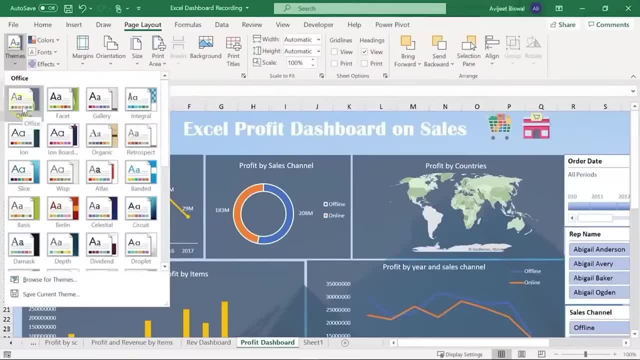 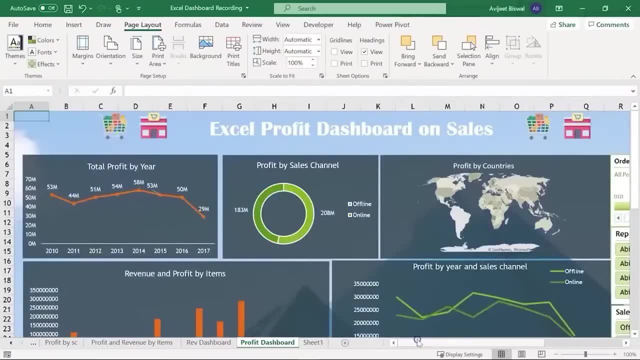 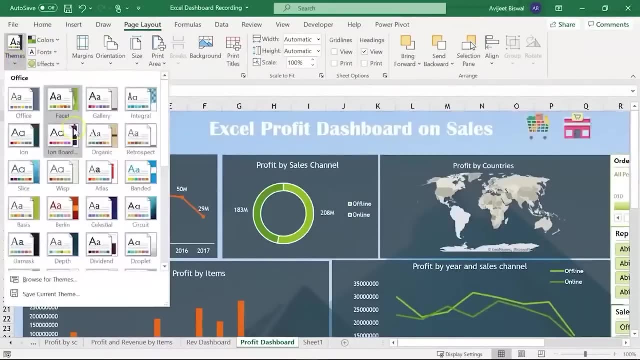 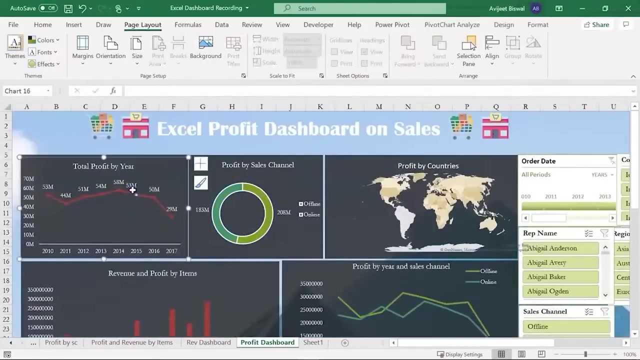 so here you can select different themes. currently we are with the office theme. now let me just select another theme. let's say facet. you see the colors have changed and it looks really beautiful. similarly, let me try out another theme. let's say organic. you see our chart has changed. let me just delete this. 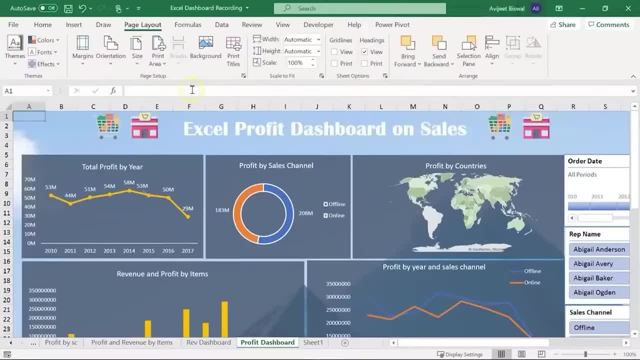 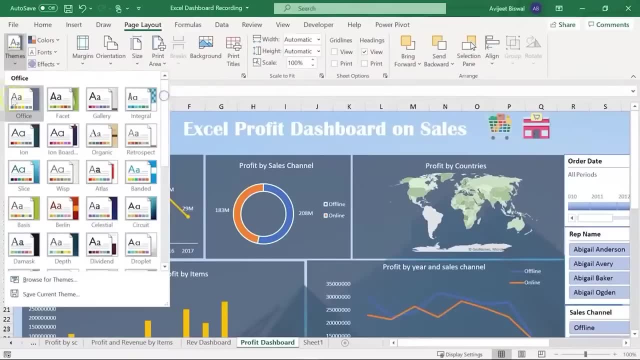 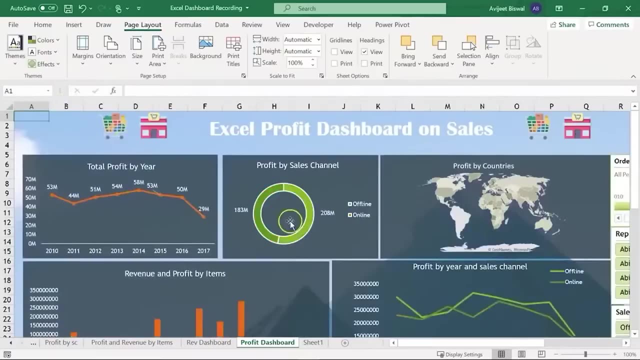 the look and feel of the dashboard by going to the page layout tab. under page layout you have themes, so here you can select different themes. currently we are with the office theme. now let me just select another theme, let's say facet. you see, the colors have changed. 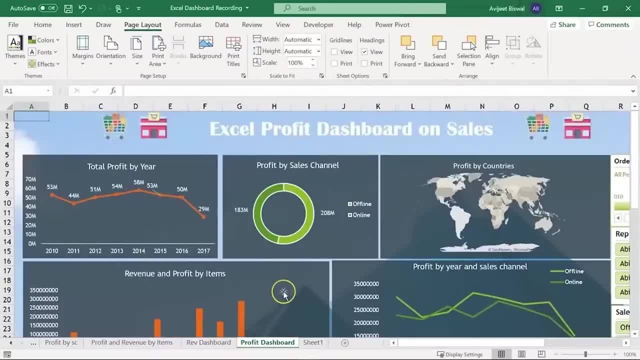 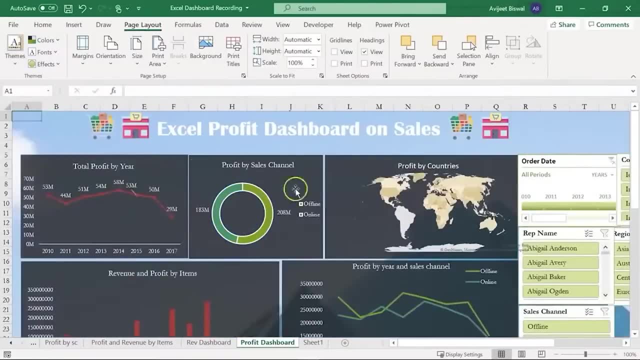 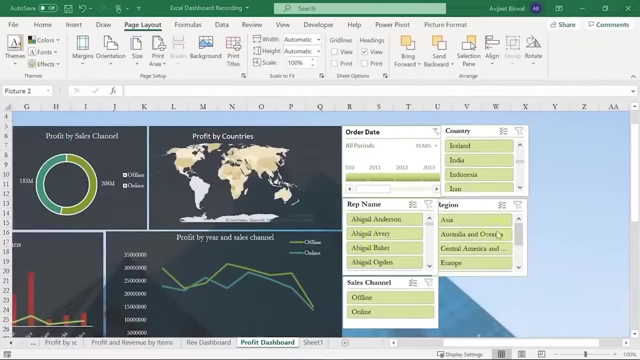 and it looks really beautiful. similarly, let me try out another theme. let's say organic. you see, our chart has changed. let me just delete this. okay, now, once you change the theme, the text also change a bit. you can see the slicers are in a different font. 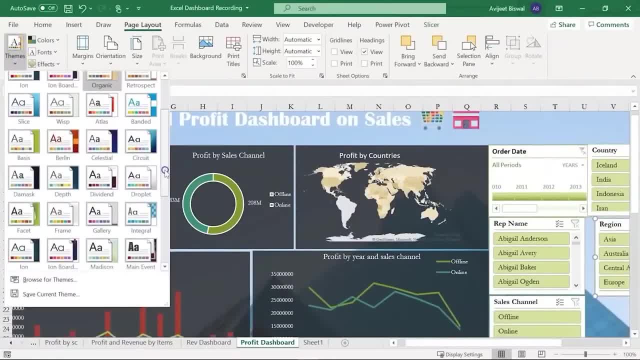 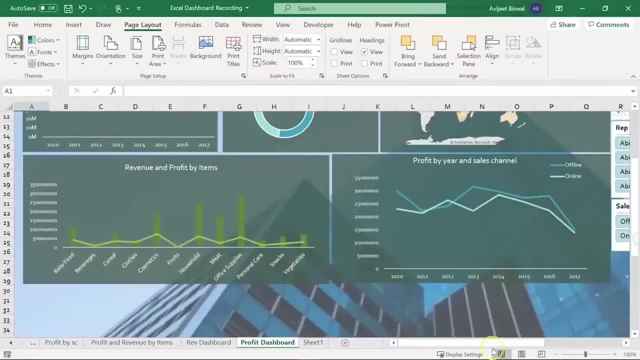 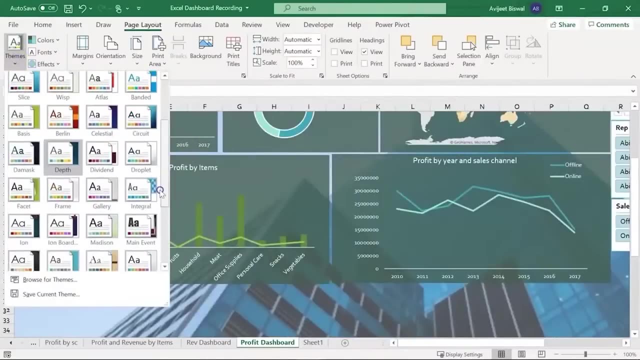 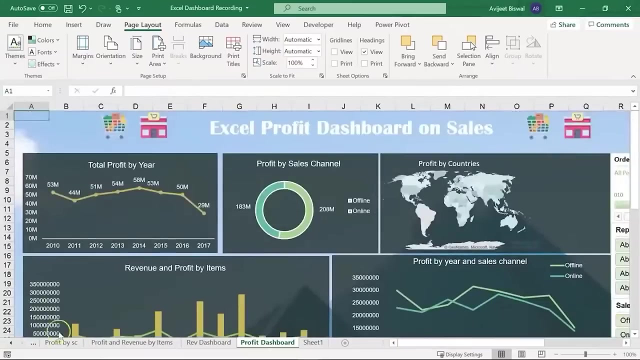 let me explore one more theme. let's say, this time I am going to choose depth, and this is more of a green type of color. you can play around and select whatever theme suits the best. alright, now let me just move back to my revenue dashboard and see. 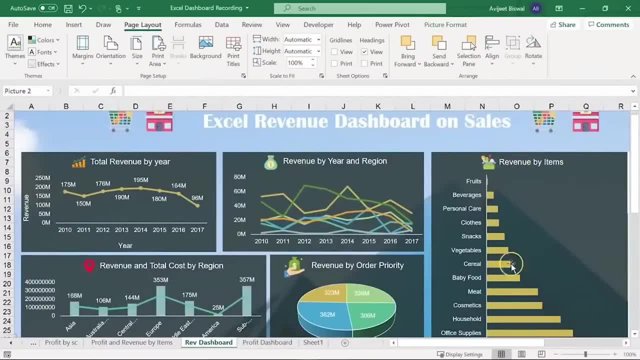 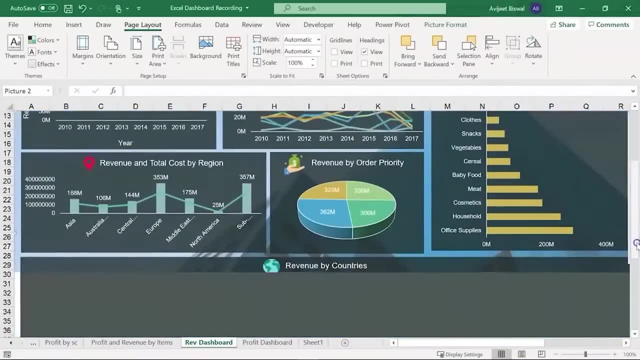 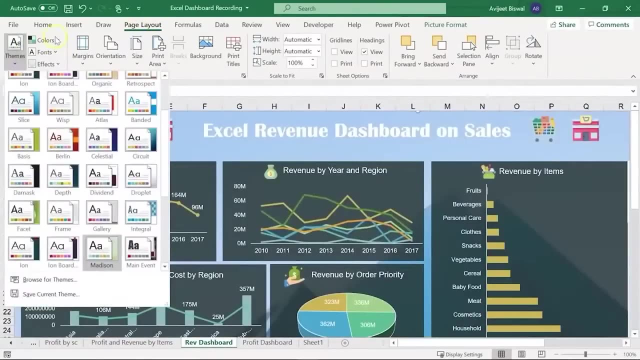 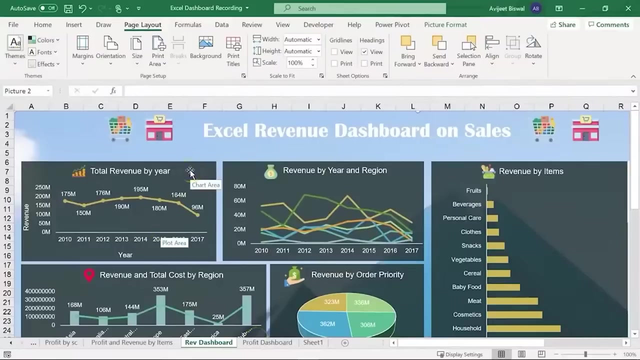 how it looks. there you go. so since we changed our theme, even our revenue dashboard is also impacted. so this is how it looks now. you can always go ahead and play with different themes, colors, fonts and effects. alright, so in this demo, we saw how to create a revenue dashboard. 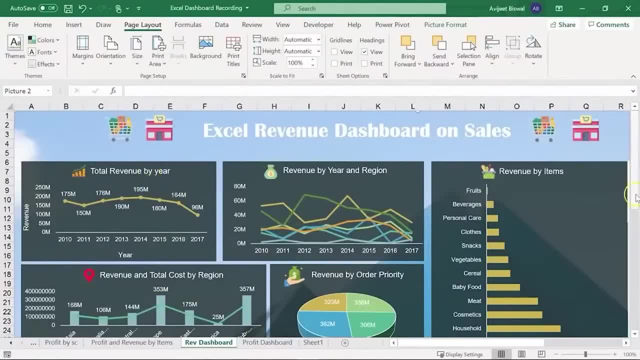 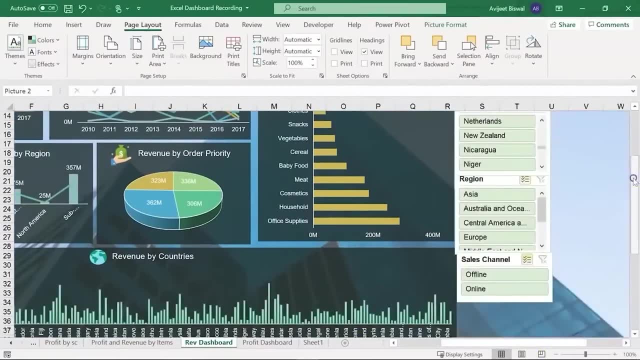 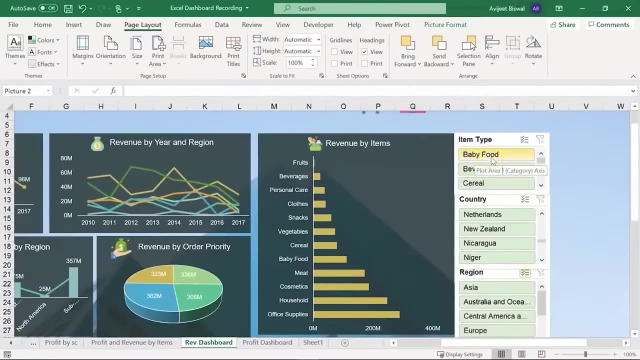 so we created line charts, this combo chart, pie chart, horizontal and vertical bar charts, and then we learnt how to add slicers and connect it to different pivot tables and we filtered our data to see revenue as well as profit, by items, by countries, by different regions, sales channel. 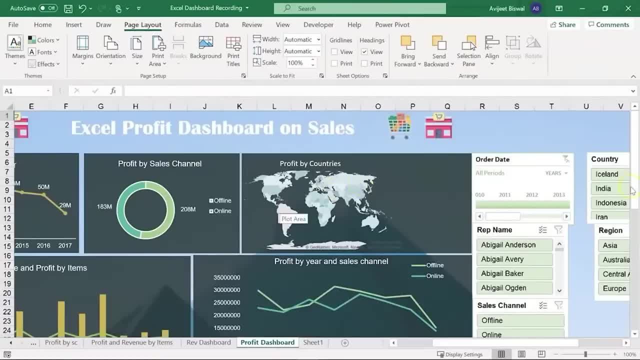 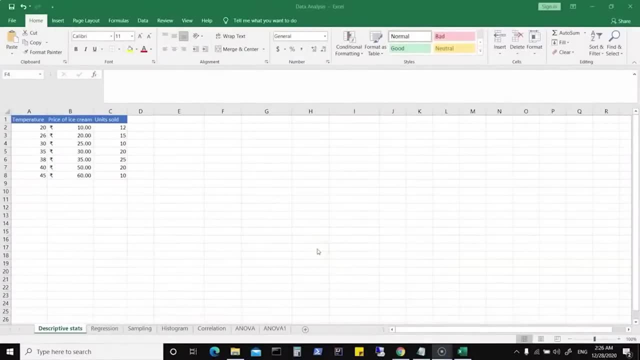 we learnt how to create a map and lots more. let's quickly see some more examples of doing data analysis using excel, and for that we can use some inbuilt add-ins which can be added to our excel sheet. so, for example, if you would want to do a descriptive, 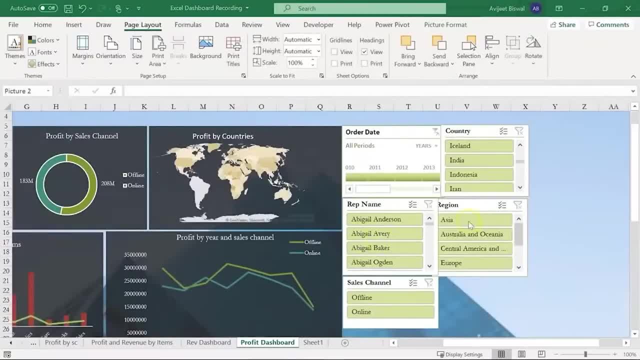 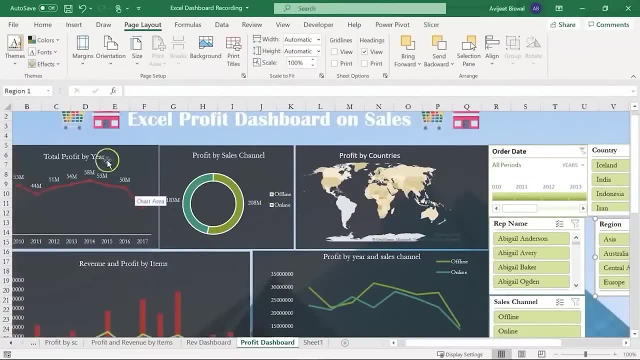 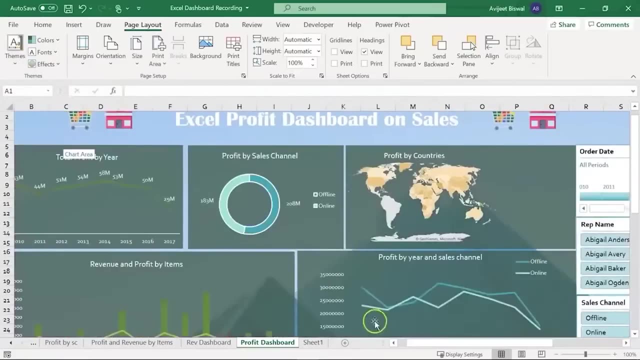 okay. so now, once you change the theme, the text also change a bit. you can see the slicers are in a different font. let me explore one more theme. let's say: this time i'm going to choose depth and this is more of a green type of color. 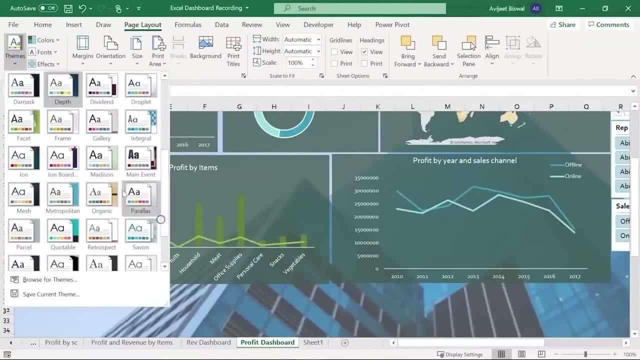 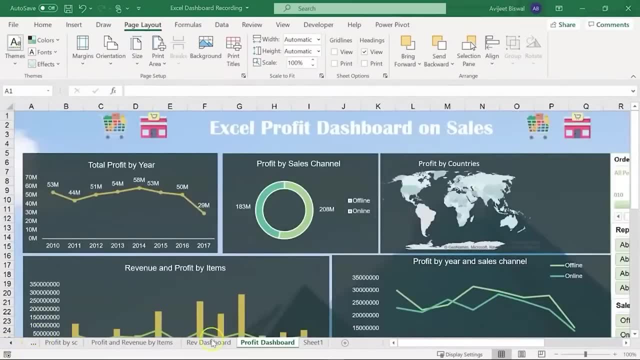 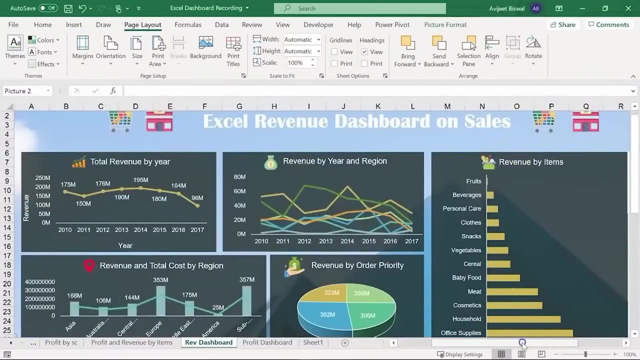 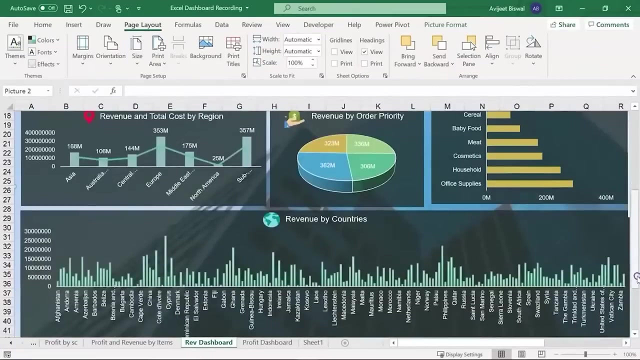 you can play around and select whatever theme suits the best. all right, now let me just move back to my revenue dashboard and see how it looks. there you go. so since we changed our theme, even our revenue dashboard is also impacted. so this is how it looks now. 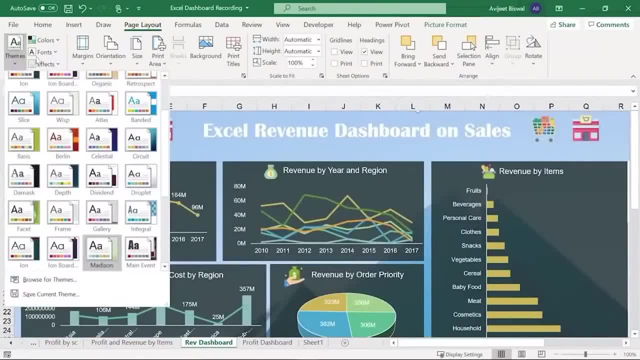 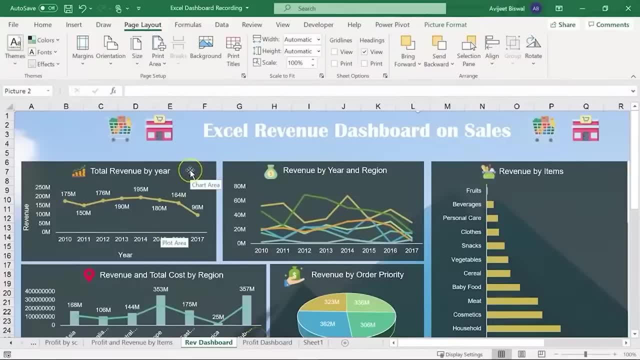 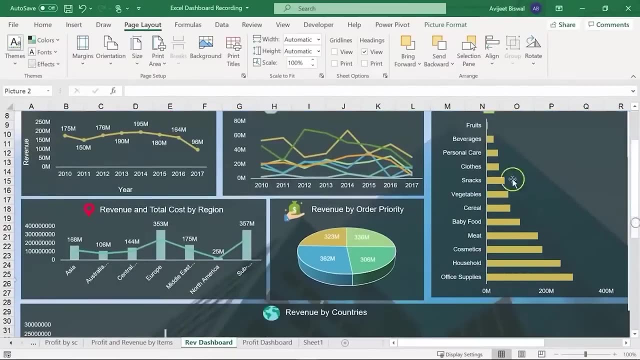 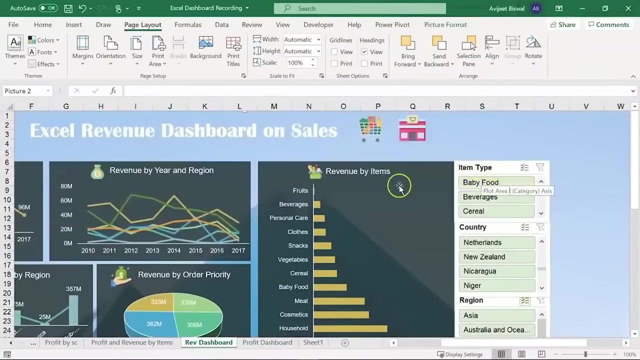 you can always go ahead and play with different themes, colors, fonts and effects, all right. so in this demo we saw how to create a revenue dashboard. so we created line charts, this combo chart, pie chart, horizontal and vertical bar charts, and then we learnt how to add slicers and connect it to different pivot tables and we filtered our 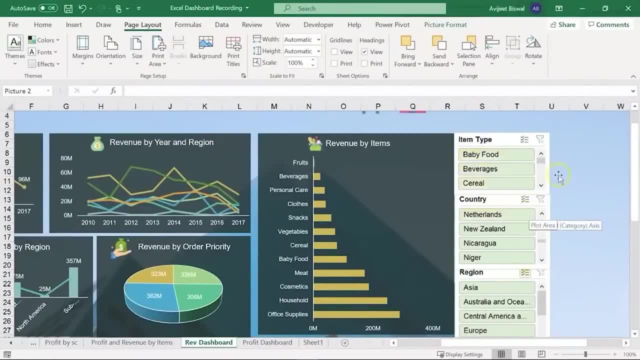 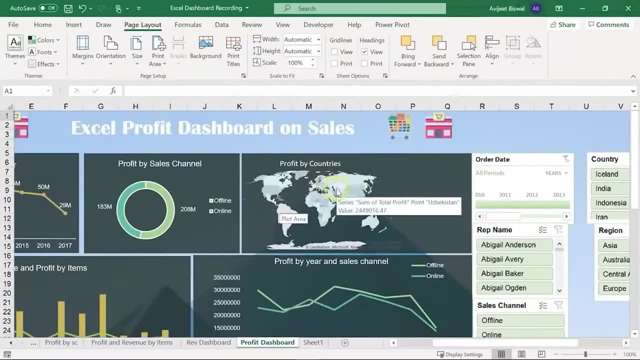 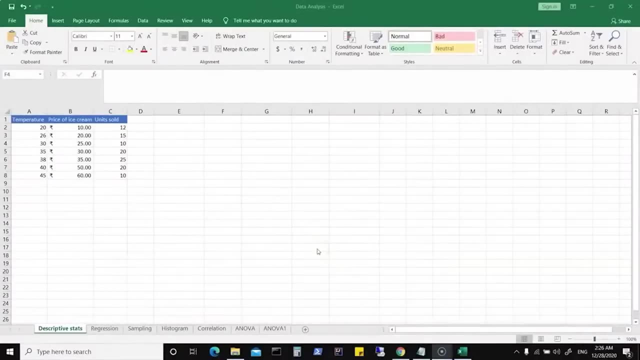 data to see how to create a revenue dashboard. so in this demo we saw how to create a revenue dashboard: revenue as well as profit by items, by countries, by different regions, sales channel. we learnt how to create a map and lots more. let's quickly see some more examples of doing data analysis using Excel, and for that we can use some. 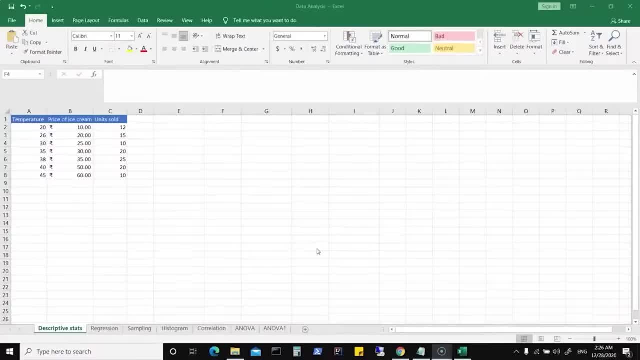 inbuilt add-ins which can be added to our excel sheet. so, for example, if you would want to do a descriptive analytics or descriptive analysis on your data- say, for example, getting your descriptive statistics such as your mean median, more and so on, so we can do that and we can use Excel for it. so for 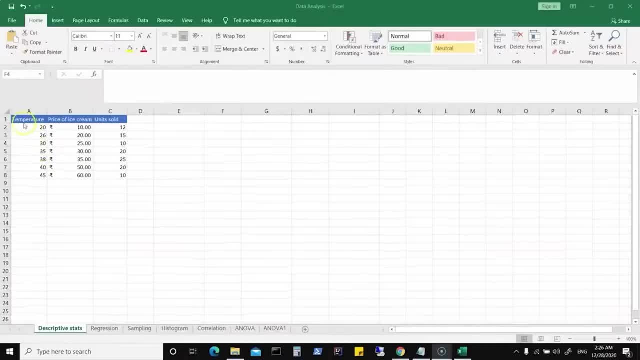 example, you can, if you are given some data. say, I have temperature price of ice cream units sold and I would want to have descriptive statistics on this. what I can do is I can click on file and you can seven. click on file and you can have a little bit more. 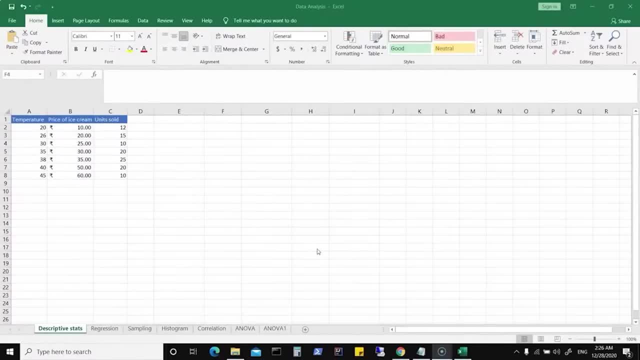 analytics or descriptive analysis on your data, say, for example, getting your descriptive statistics such as your mean median mode and so on. so we can do that and we can use excel for it. so, for example, you can, if you are given some data, say: I have temperature, price of ice. 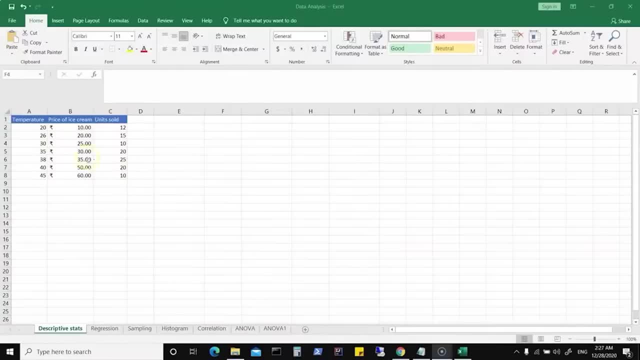 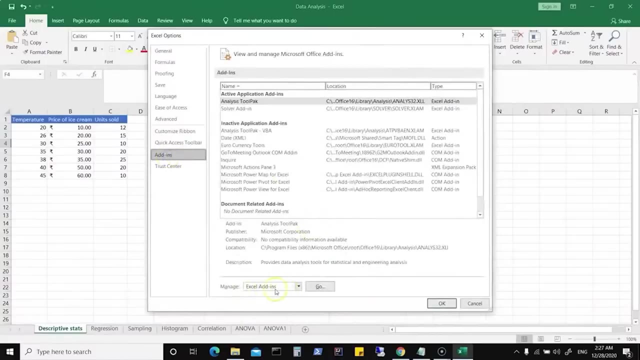 cream units sold and I would want to have descriptive statistics on this. what I can do is I can click on file and here in file you can click on options and within options, click on add-ins. now, within add-ins, you have excel add-ins, which is selected here, so click. 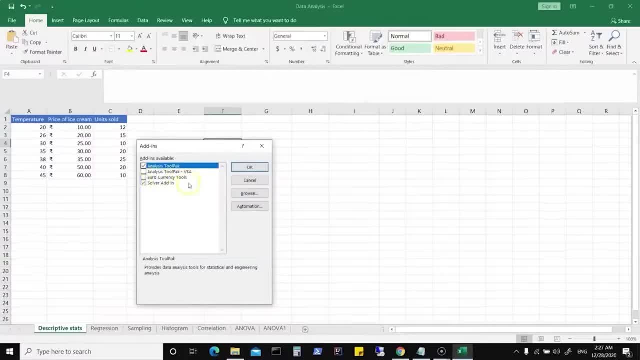 on, say go, for example, and that shows what add-ins are available and you can choose which ones are you interested in. so for example, I have chosen analysis tool pack and solver add-in and click on ok. now that basically should add more options to your excel. so if you click on data, 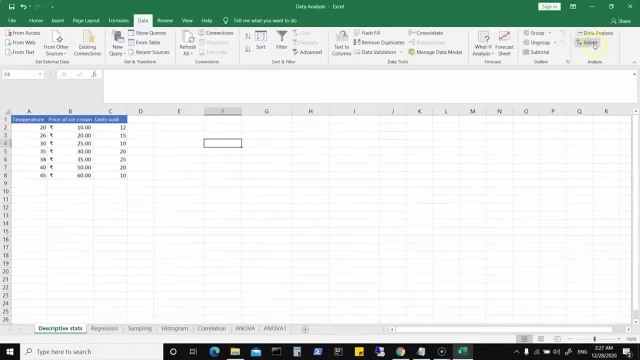 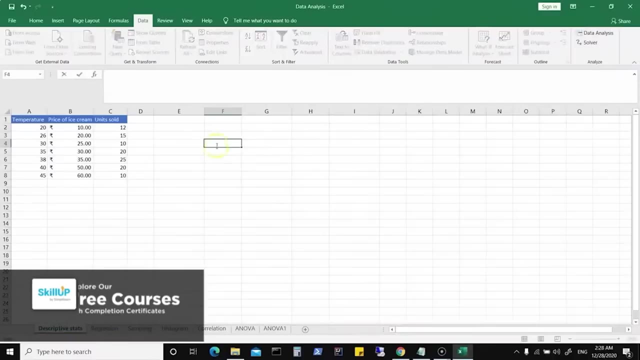 so here you see data analysis and solver, and this is what we would want to use to get our descriptive statistics for these three columns. so, for example, let's say temperature, or you can even give the names later, once you get your descriptive statistics. so, for example, let's go for data analysis. 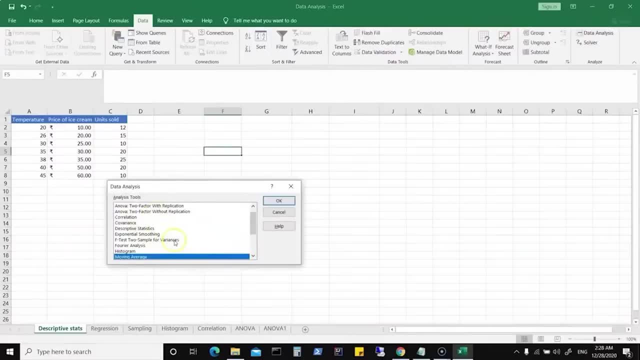 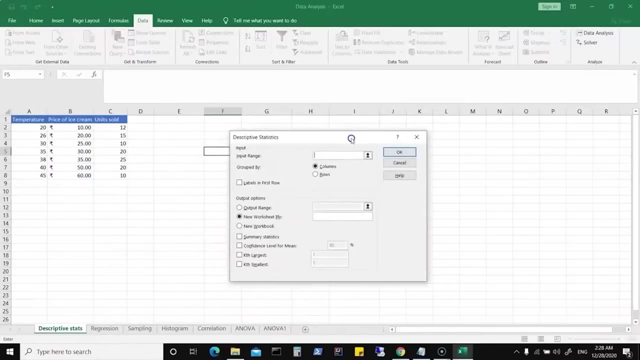 and here it says: what are you interested in? there is a two factor with replication. you have correlation, covariance, descriptive statistics. you have histogram, so let's click on descriptive statistics, click on ok. now this one basically asks your input range. so, while your cursor is blinking, here also. 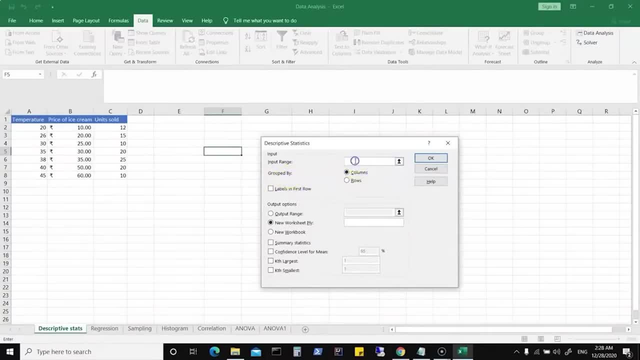 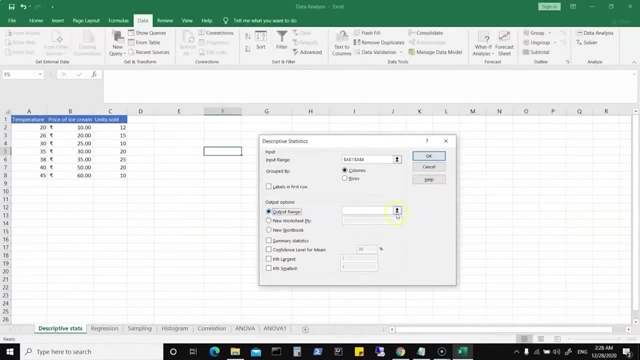 it is said grouped by, so let's give it a range. so, for example, I will say, say temperature. now, if I do this and I have selected the heading, just look at that. and now you need an output range. so let's just select this and then you can have your cursor blinking. 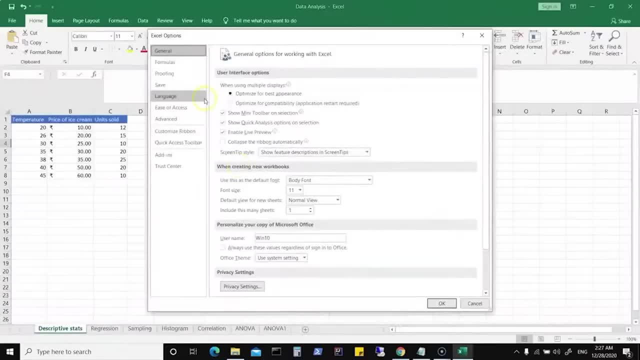 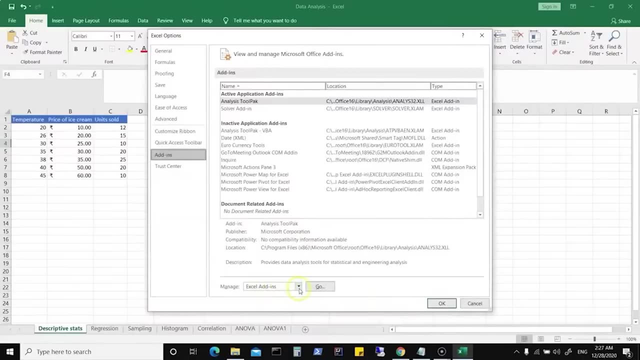 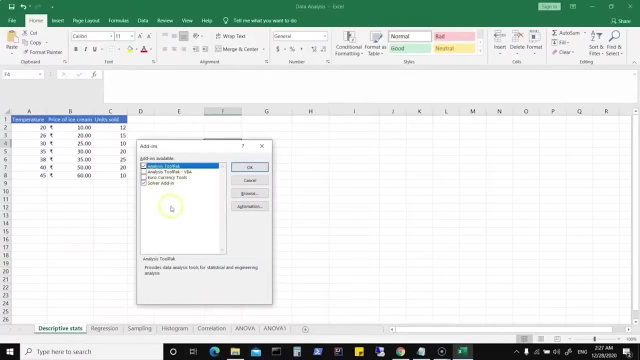 And here in file you can click on options and within options click on add-ins. Now, within add-ins you have Excel add-ins, which is selected here. So click on say go, for example, and that shows what add-ins are available and you can choose which ones are you interested in. 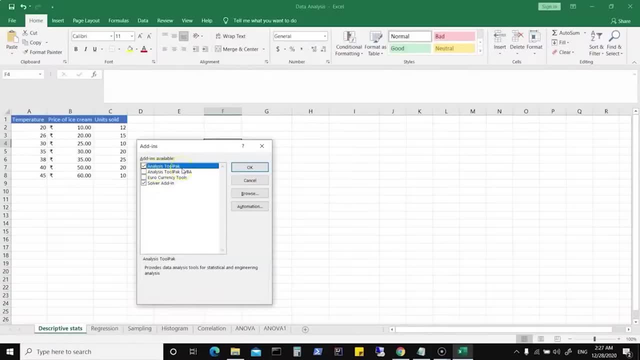 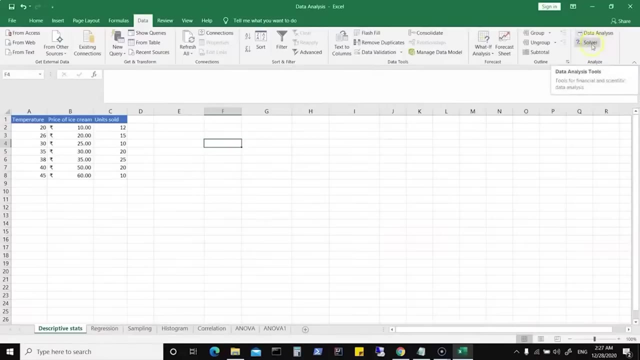 So, for example, I have chosen analysis tool pack and solver add-in and click on OK. Now that basically should add more options to your Excel. So if you click on data, so here you see data, analysis and solver, And this is what we would want to use to get our descriptive statistics for these three columns. 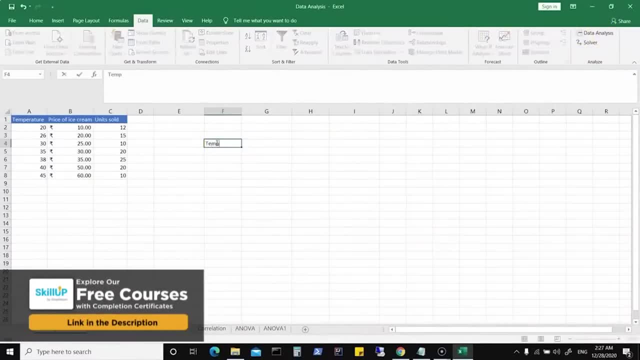 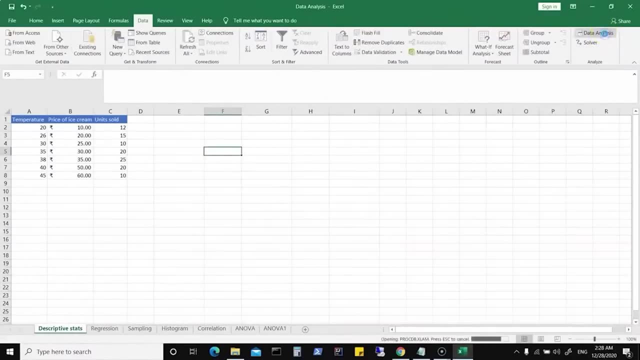 So, for example, let's say temperature, or you can even give the names later, once you get your descriptive statistics. So, for example, let's go for data analysis And here it says: what are Are you interested in? There is a two factor with replication. 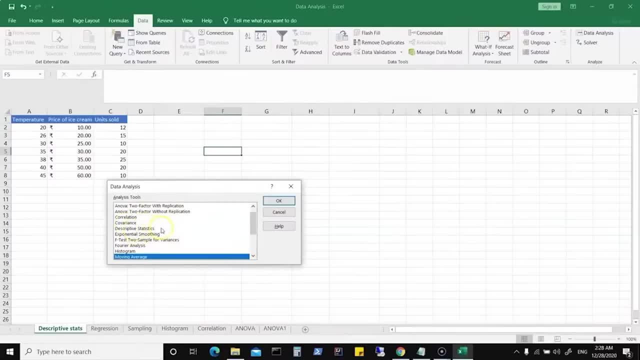 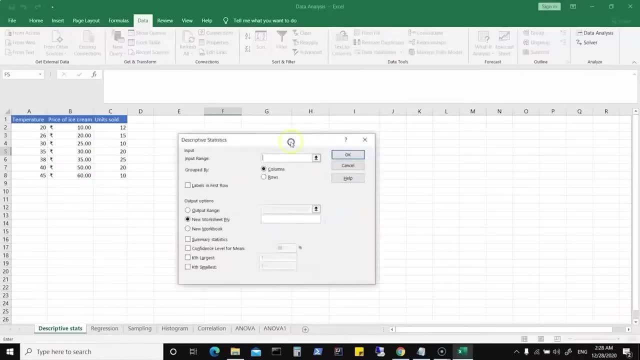 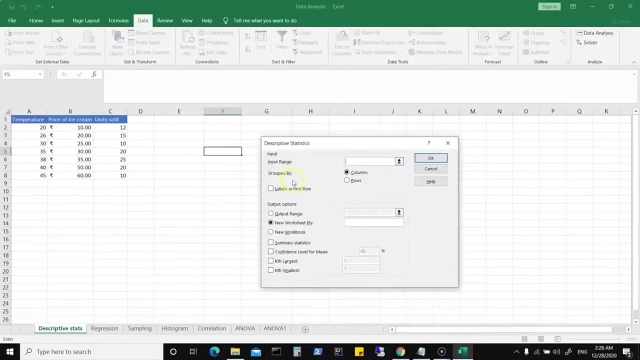 You have correlation covariance, descriptive statistics, You have histogram, So let's click on descriptive statistics. Click on OK. Now this one basically asks your input range. So while your cursor is blinking, here also it is said grouped by, So let's give it a range. 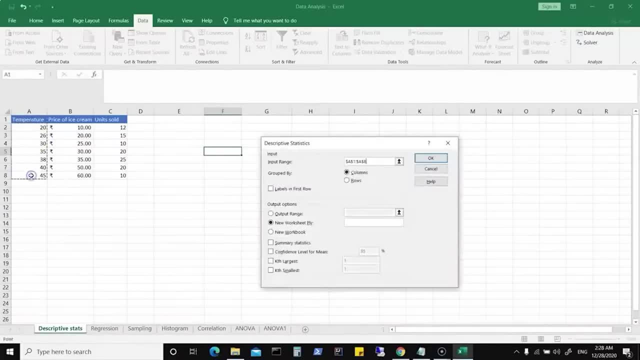 So, for example, I will say, say temperature Now. Now, if I do this and I have selected the heading, just look at that. and now you need an output range. So let's just select this and then you can have your cursor blinking here. 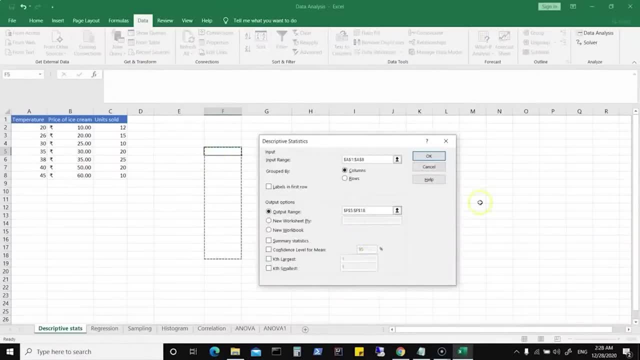 Let's select, say, fields here, And this is where I would want the output. Now. it also said what options do you want? So it has output range. We can then select summary statistics, confidence level. So I will say summary statistics is what I'm interested in. 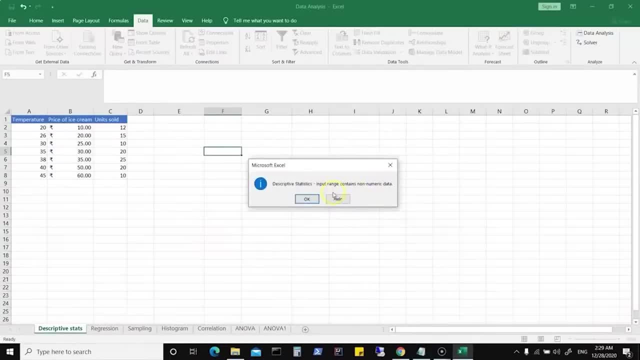 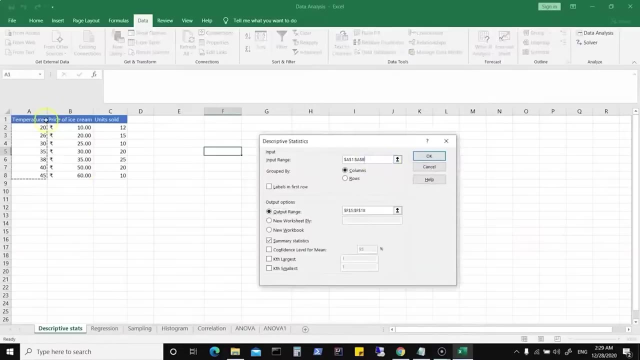 Say OK and this says input. input range contains non-numeric data. Now, why is that? Because we chose temperature, the heading also, So click on OK And here we will alter the range. So this one is our range should be only the values, numeric values, on which we would want the descriptive statistics. 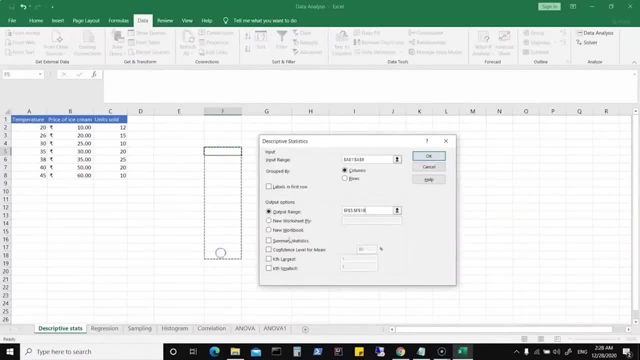 here. let's select, say, fields here, and this is where I would want the output. now it also said what options do you want? so it has output range. we can then select summary statistics, confidence level. so I will say summary statistics is what I am interested in, say ok. 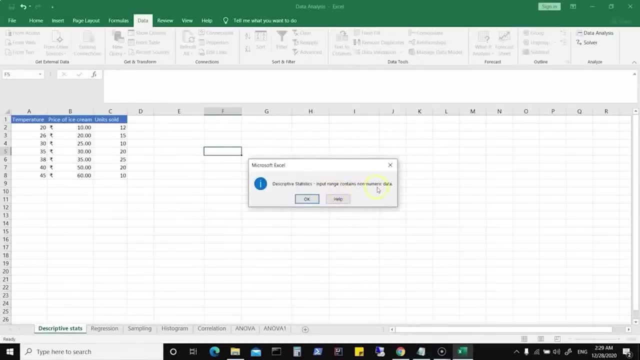 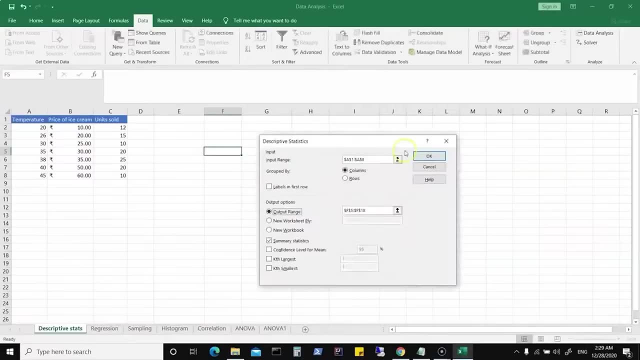 and this says input. input range contains non numeric data. now, why is that? because we chose temperature, the heading also, so click on ok and here we will alter the range. so this one is our range should be only the values, numeric values- on which we would want the descriptive statistics. 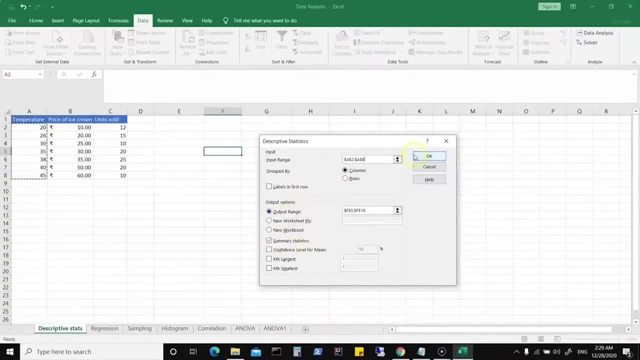 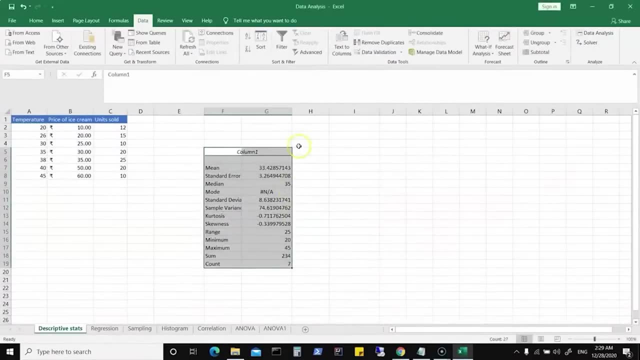 we have output range already selected, we have summary statistics and now you can click on ok and that basically gives your descriptive statistics for temperature. so here I could basically given a value for this so I can say temperature and that's my descriptive statistics for temperature might be. I can just 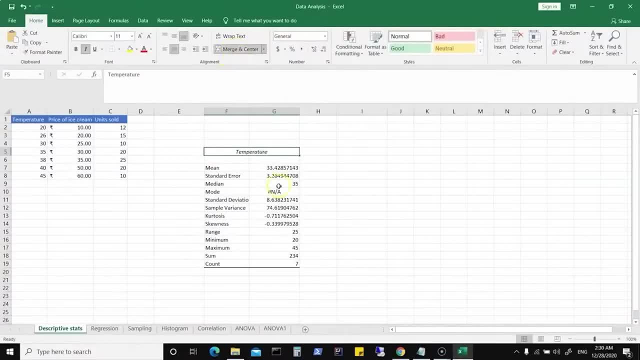 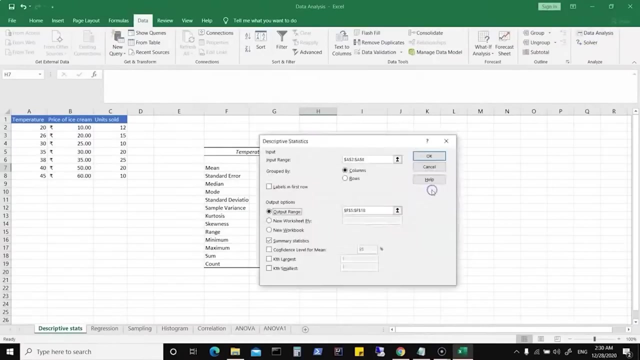 do some formatting and that's it. so that gives me descriptive statistics for the values here. now, similarly, we can do it for price of ice cream. so what we need is we need to basically go for data, data analysis. descriptive statistics say: ok, now you need to give a range. so here, 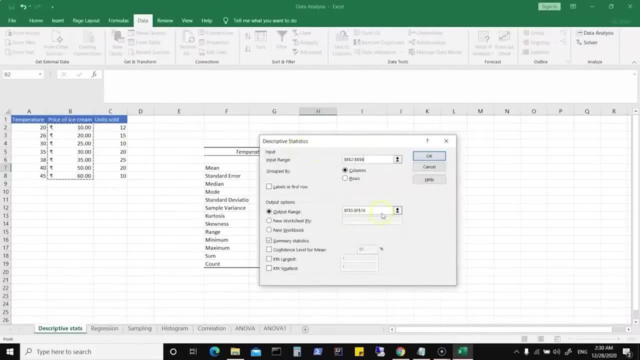 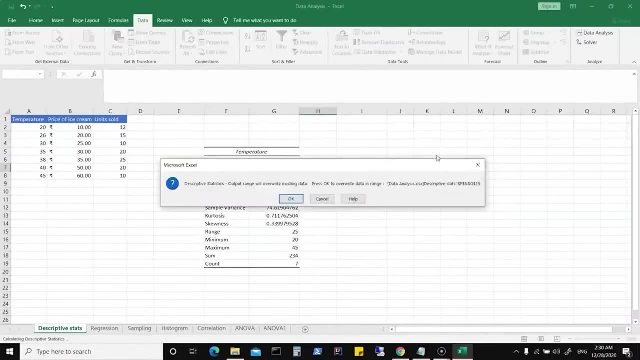 I will change my range to these values. output range is already selected. now we are interested in summary statistics. click on ok and this says output range will overwrite existing data. press ok to overwrite data in range. I will say cancel. no, that's not what we want to do. we need to. 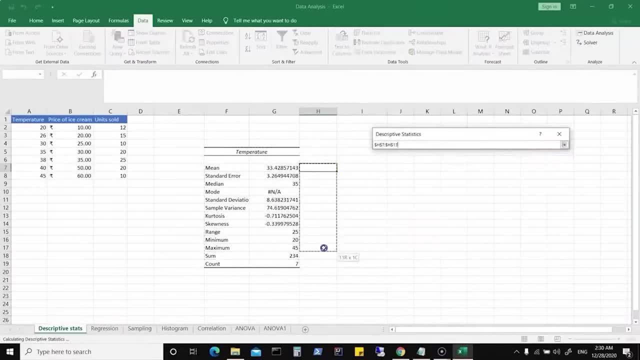 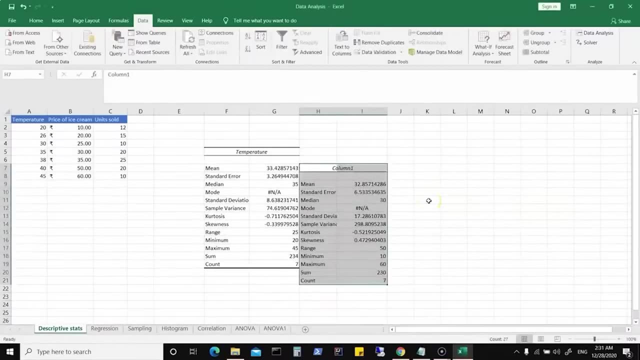 give a new range. so let's select our new range, which is here and now click on ok, so now we get the values, which is for your price of ice cream. so again, we can basically select this and say price of ice cream and we got our descriptive statistics. 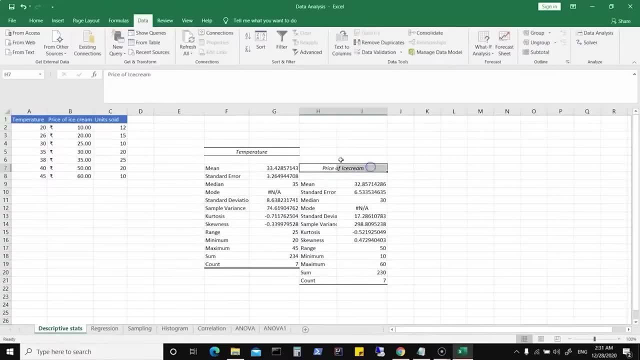 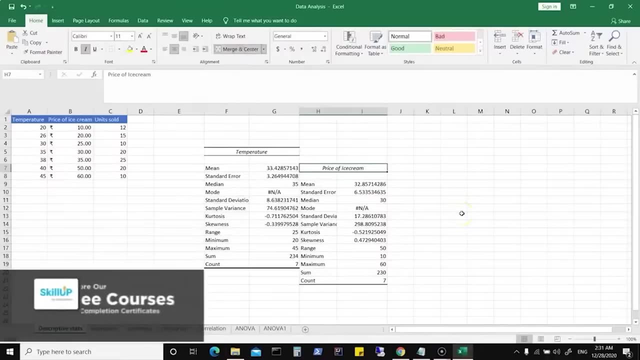 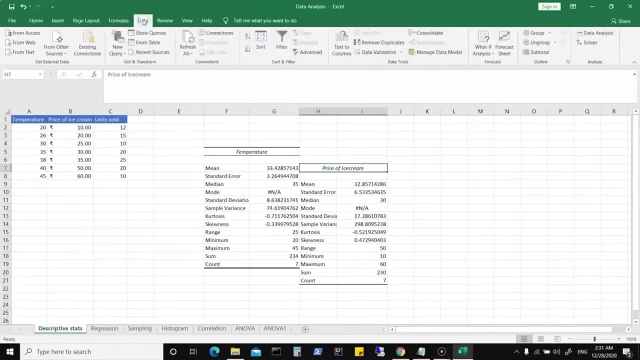 for price of ice cream and, like we did earlier, I can select this. I can basically do a merge and center and that gives me descriptive statistics for price of ice cream, so we could also basically change this. now I can go into data and I can go into data. 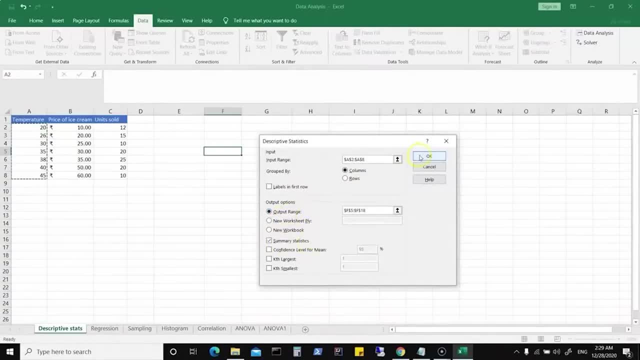 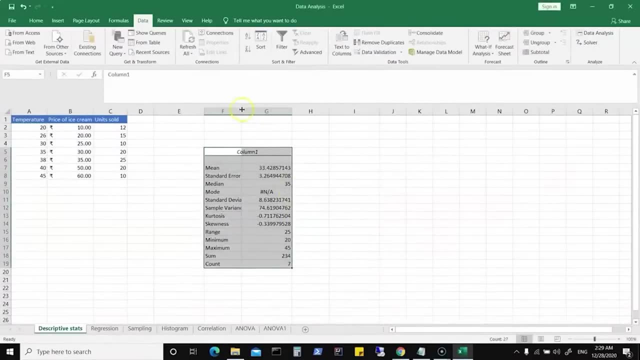 We have output range already selected, We have summary statistics And now you can click on OK And that basically gives your descriptive statistics for temperature. So here I could basically given a value for this, So I can say temperature and that's my descriptive statistics for temperature. 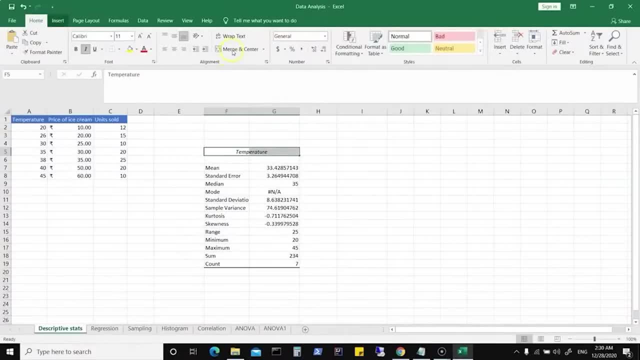 Might be. I can just do some formatting and that's it. So that gives me descriptive statistics for the values here. Now. similarly, we can do it for price of ice cream. So what we need is we need to basically go for data. 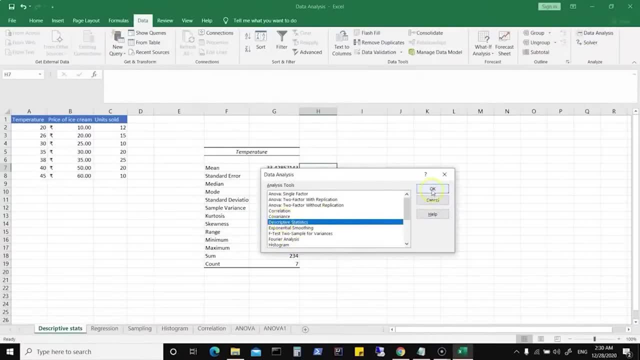 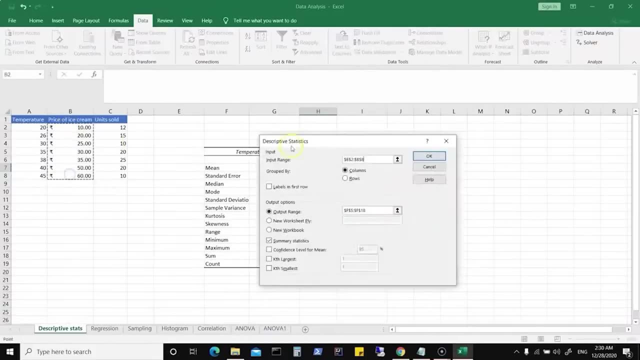 Data analysis. descriptive statistics say OK, now you need to give a range. So here I will change my range to these values. Output range is already selected. Now we are interested in summary statistics. Click on OK And this says output range will overwrite existing data. 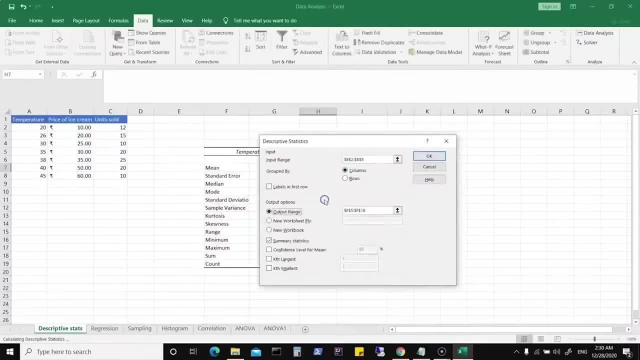 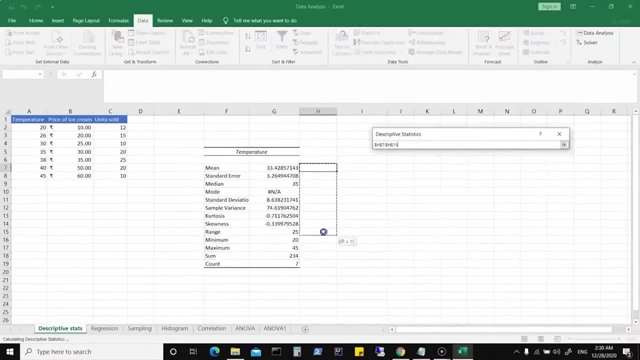 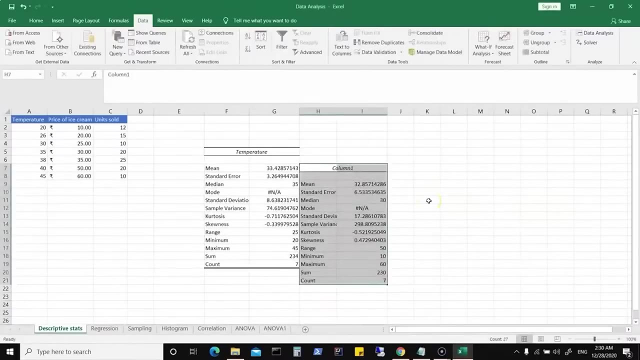 Press OK to overwrite data in range, I will say cancel. No, that's not what we want to do. We need to give a new range. So let's select our new range, which is here, And now click on OK. So now we get the values, which is for your price of ice cream. 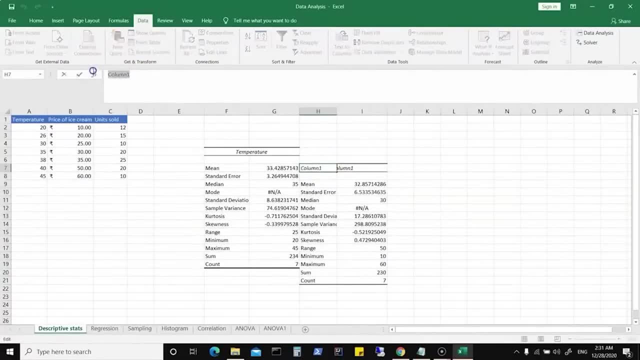 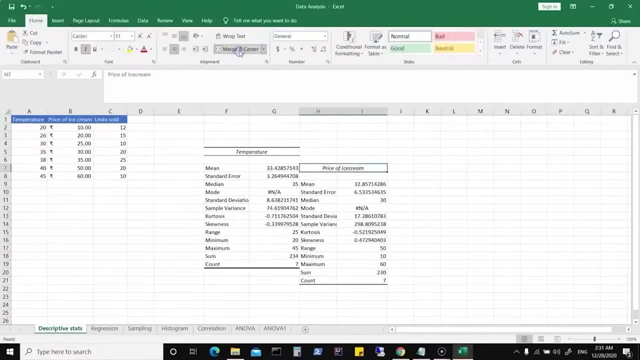 So again, we can basically select this And say price of ice cream, And we got our descriptive statistics for price of ice cream And, like we did earlier, I can select this. I can basically do a merge and center And that gives me descriptive statistics for price of ice cream. 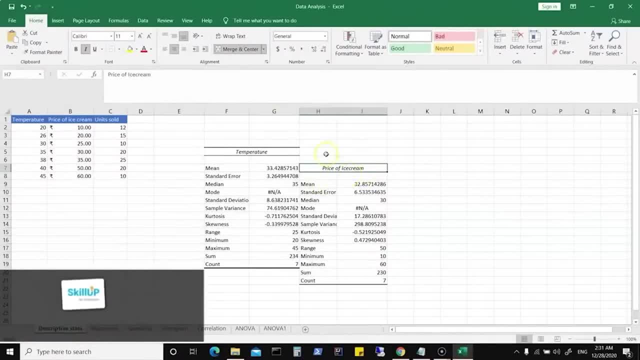 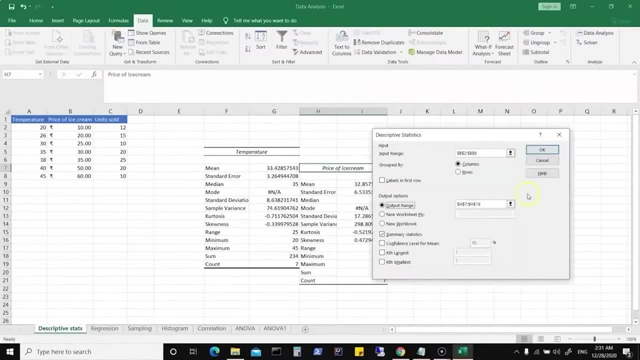 So we could also basically change this. Now I can go into data and I can go into data analysis, descriptive statistics. So we know that we had selected this B2 to B8. And this one which is H6 to H19,. 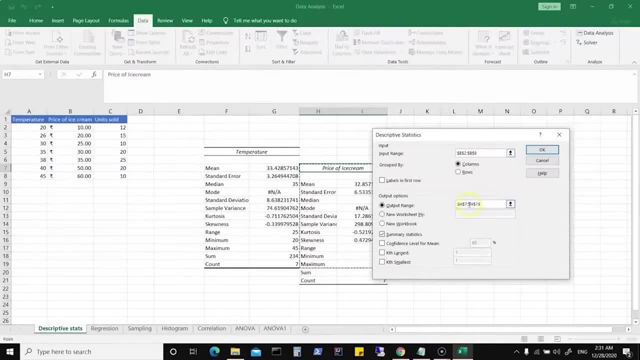 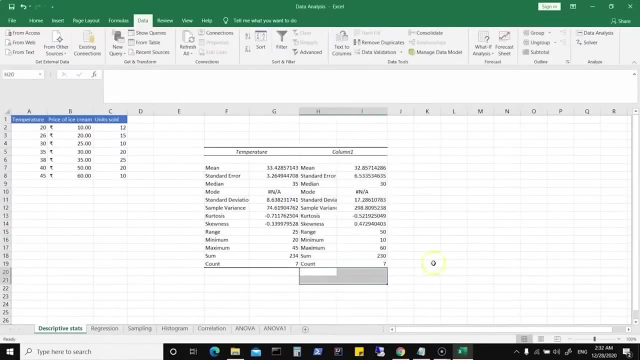 we would want to shift. it might be two columns up, So might be. I can just say H5. And I can manually change it to H17. And let's say OK, And we will basically get this And I can get rid of this. 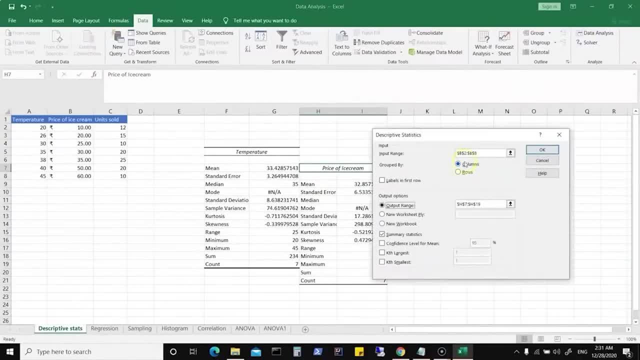 analysis descriptive statistics. so we know that we had selected this b2 to b8 and this one which is h6 to h19. we would want to shift. it might be two columns up, so might be. I can just say h5 and I can manually change it to h17. 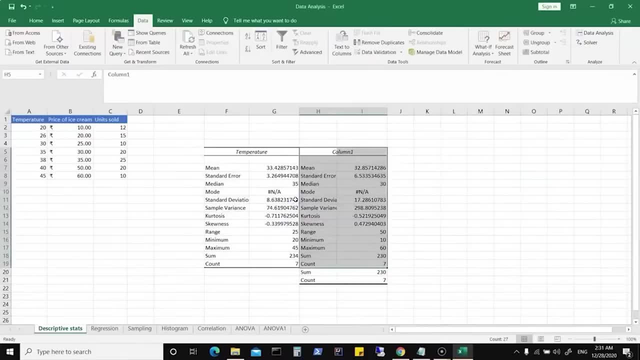 and let's say ok, and we will basically get this and I can get rid of this, so I can have it in the same range, so similarly. so this one will have to be renamed and I can basically say: price of ice cream, and that's basically my. 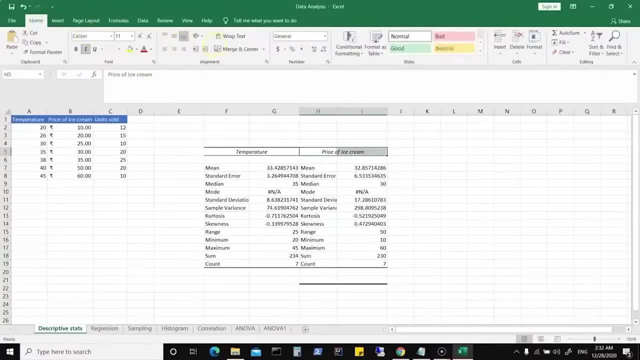 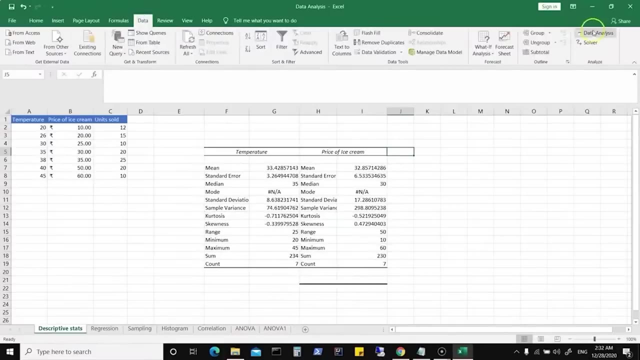 descriptive statistics for my price of ice cream, and similarly we can do it for the third column, which is units sold. so we would want to have this. now. let's see. we can click on data, we can click on data analysis- descriptive statistics. so we need to give the range correctly. 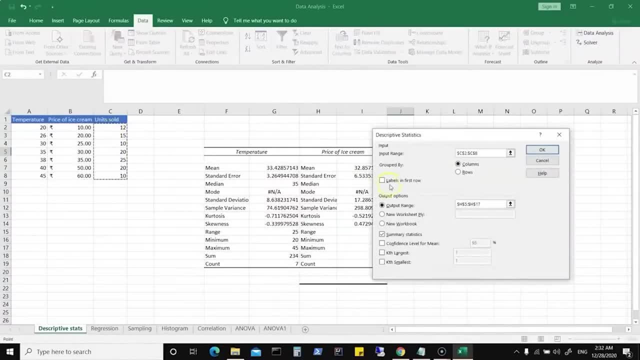 so this time our range changes to units sold. now we can also say labels in first row. ok, if we were selecting the heading, so let's do it in this way. so in my range, in my range, let me empty this- I can basically select this: which we 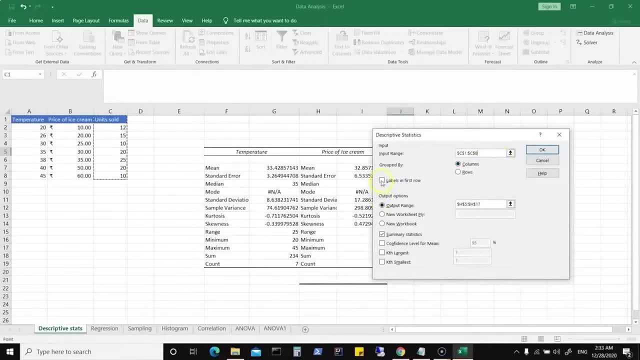 know, has non numeric data in the first row, say, for example, I'll say labels in first row. I'm interested in summary statistics- and this range will now have to be changed from H to basically something like J. so let's say J and let's select these. 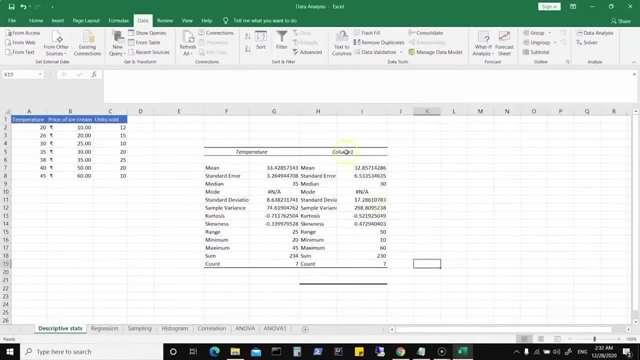 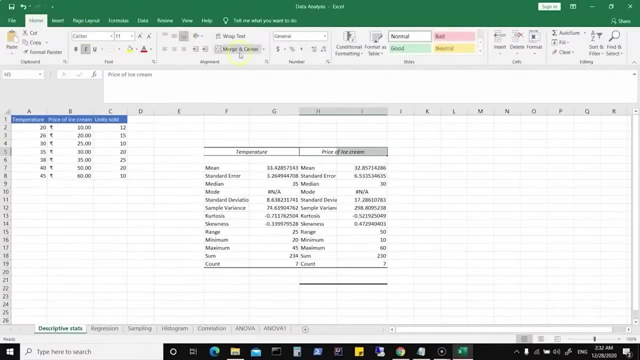 So I can have it in the same range, So similarly. so this one will have to be renamed And I can basically say price of ice cream, And that's basically my descriptive statistics for my price of ice cream. And similarly we can do it for the third column, which is units sold. 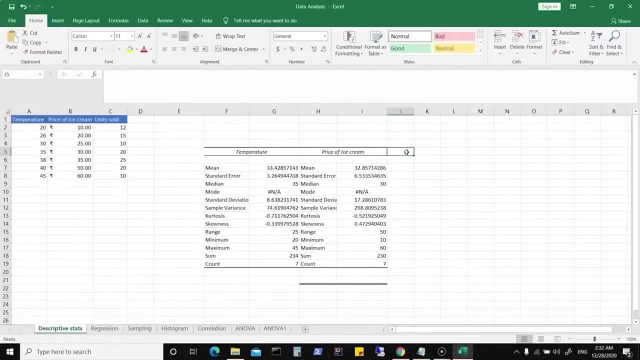 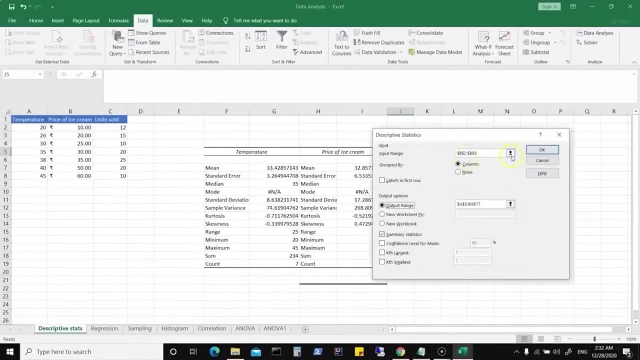 So we would want to have this. Now, let's see, we can click on data. We can click on data analysis, Descriptive statistics. So we need to give the range correctly. So this time our range changes to units sold. Now we can also say labels in first row. 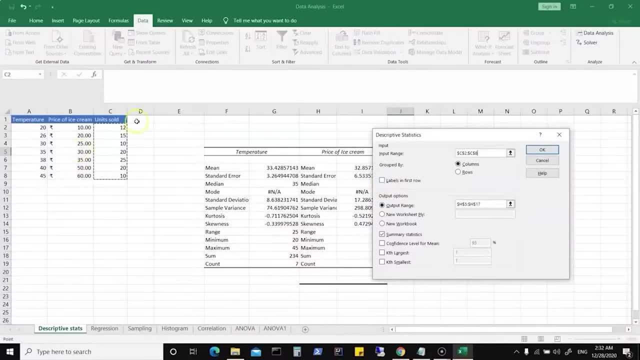 OK, if we were selecting the heading, So let's do it in this way. So in my range, in my range, let me empty this. I can basically select this, which we know has non-numeric data, in the first row. 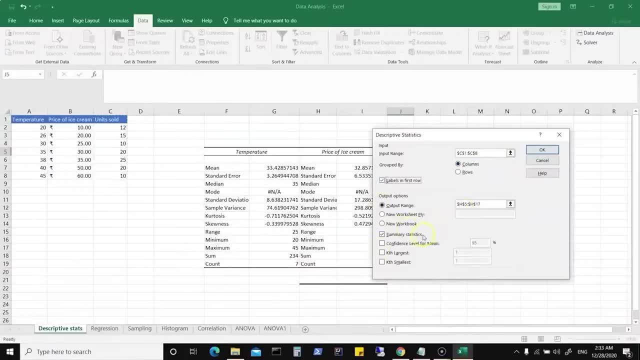 Say, for example- I'll say labels in first row- I'm interested in summary statistics- And this range will now have to be changed from H to basically something like J. So let's say J And let's select these values, So that should take care of things. 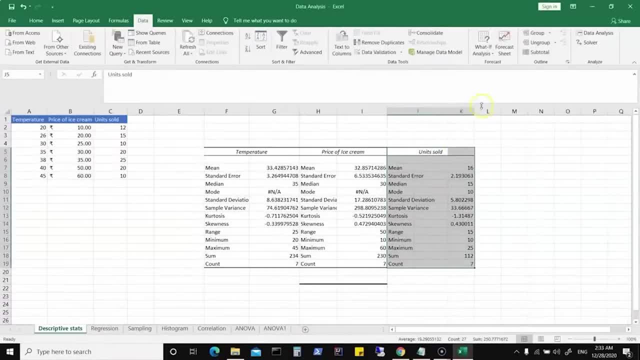 And now you see you have your units sold. You did not have to manually rename it And you have basically got the display. So that's good Descriptive statistics. So this is how you can simply perform analysis using data analysis. here You can basically get your descriptive statistics for your columns. 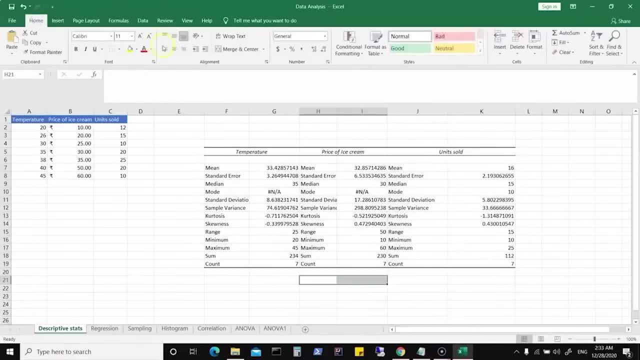 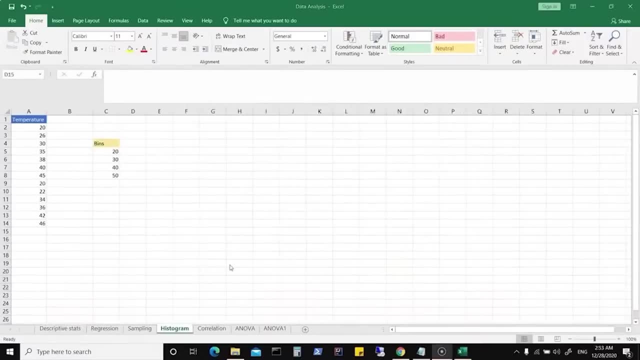 And then you can do whatever needed formatting you need to basically make your data look in a good way. Now let's look at one more example of data analysis, where we may want to look at the frequency of values, Or frequency of values occurring in a range of values. 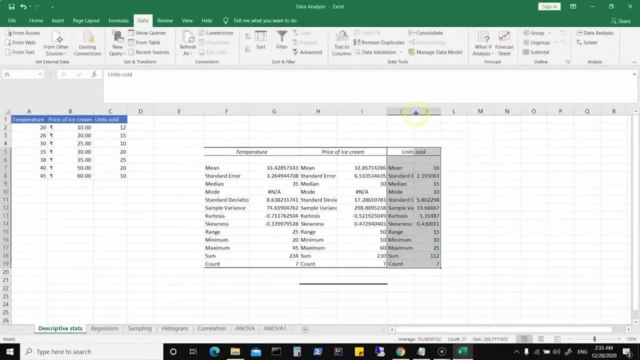 values. so that should take care of things. and now you see, you have your units sold, you did not have to manually rename it and you have basically got the descriptive statistics. so this is how you can simply perform analysis using data analysis. here you can basically get your descriptive. 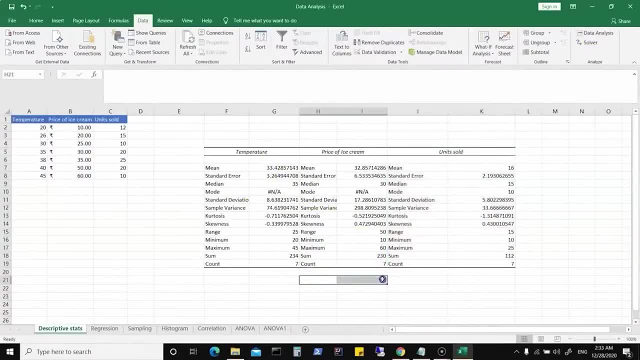 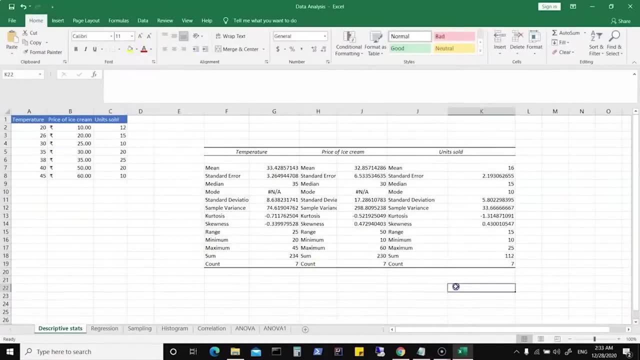 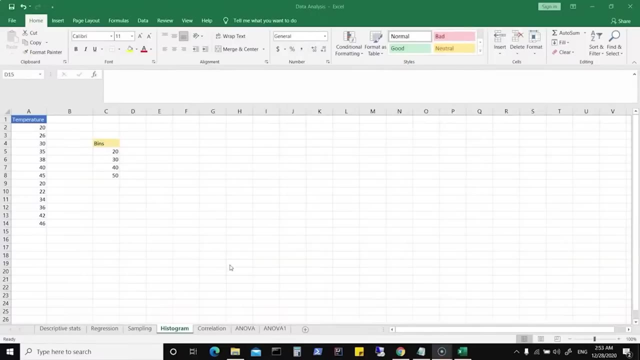 statistics for your columns, and then you can do whatever needed formatting. you need to basically make your data look in a good way. now let's look at one more example of data analysis, where we may want to look at the frequency of values, or frequency of values occurring in a 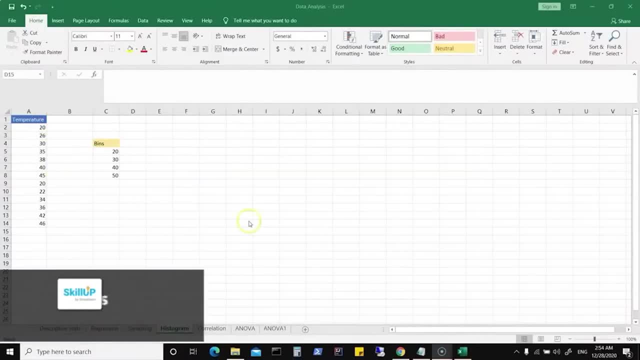 range of values. so, for example, if you have been given temperatures, you have been given some pins where you would want to identify how many values fall into the range of 0 to 20,, 20 to 30, 30 to 40,, 40 to. 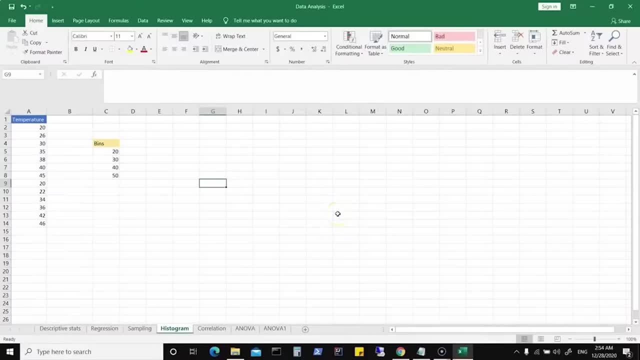 50, and the easiest way to do that would be creating histogram. now, histogram is usually used for data analysis, where you would want to look at different variables or, say, features. for example, temperature is one such feature might be. there might be one more variable or feature, such as sale of ice cream. 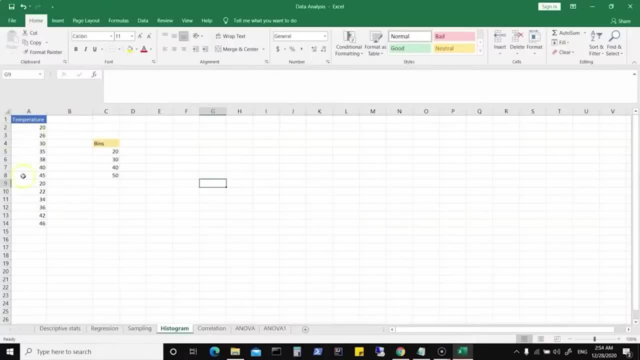 and you would want to see if the increase or decrease in temperature affects the increase or decrease in sale of ice cream might be. sale of ice cream is a response based on temperature, so it depends. so sometimes you may want to find a relationship between two variables, whether they are positively or. 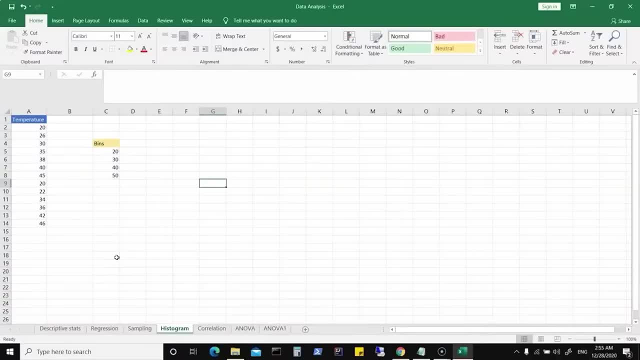 negatively related, or you would want to do different kind of analysis and in certain cases we may want to first do analysis on one single variable. look at the frequency of values might be also look at the defects and for which we can use something like Pareto chart. so we can 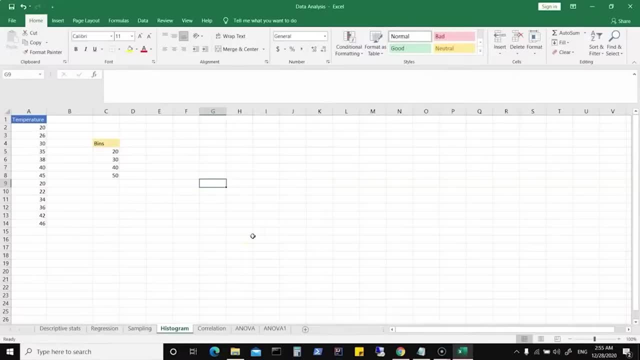 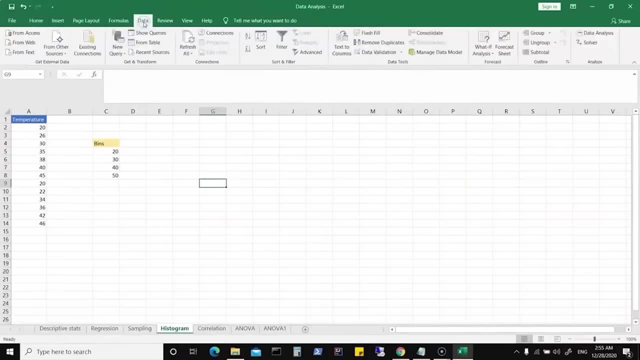 go for histogram, and that basically gives us the frequency of values. now, how do we do that? so we have already added the add-in, which is data analysis, so we can just use the same thing again here. we would want to create a histogram, so let's say okay now. 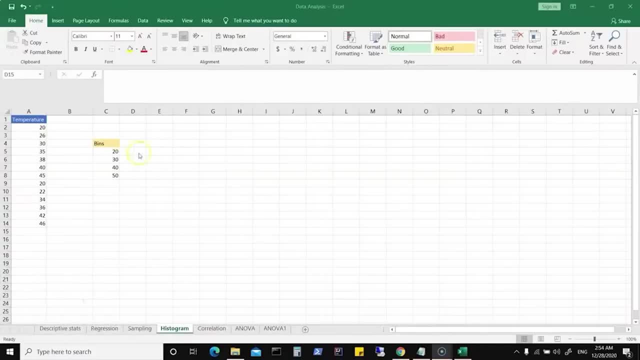 So, for example, if you have been given temperatures, you have been given some pins where you would want to identify how many values fall into the range of 0 to 20,, 20 to 30,, 30 to 40,, 40 to 50.. 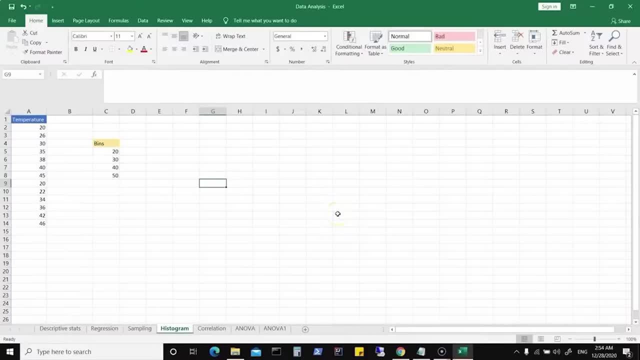 And the easiest way to do that would be creating histogram. Now, histogram is usually used for data analysis, Where you would want to look at different values. You would want to look at different variables or, say, features. For example, temperature is one such feature. 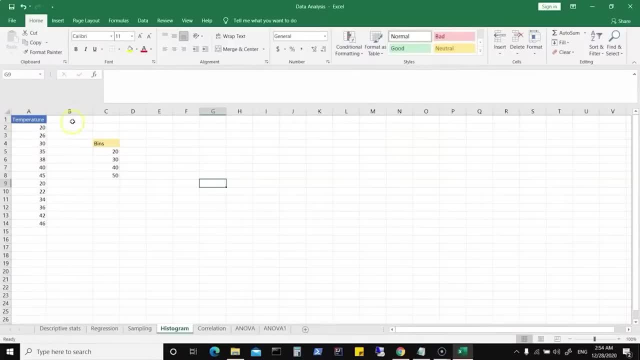 There might be one more variable or feature, such as sale of ice cream, And you would want to see if the increase or decrease in temperature affects the increase or decrease in sale of ice cream Might be. sale of ice cream is a response based on temperature. 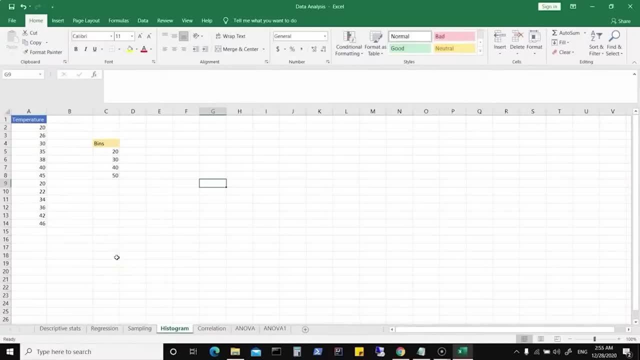 So it depends. So sometimes you may want to find a relationship between two variables, Whether they are positively or negatively related, Or you would want to do different kind of analysis And in certain cases we may want to first do analysis on one single variable. 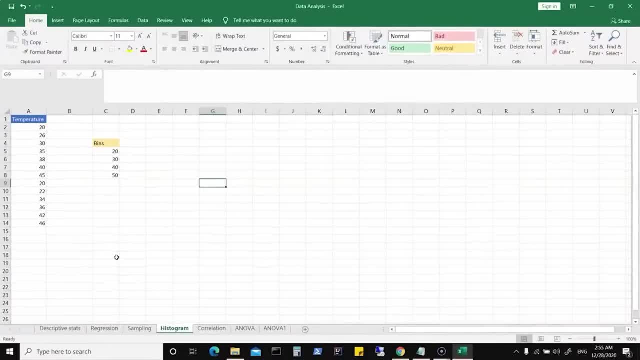 Look at the frequency of values, Might be also look at the defects And for which we can use something like Pareto chart, So we can go for histogram And that basically gives us the frequency of values. Now, how do we do that? 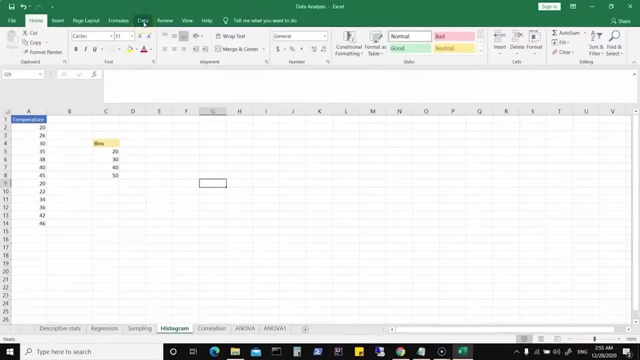 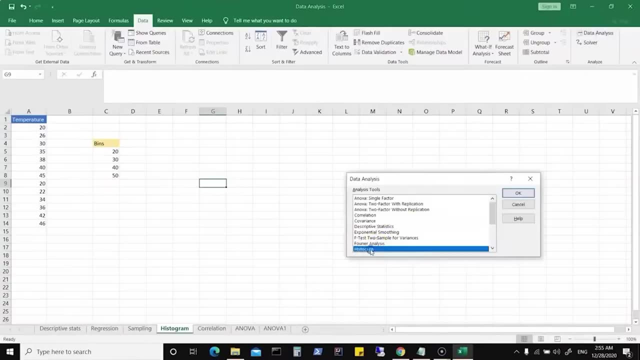 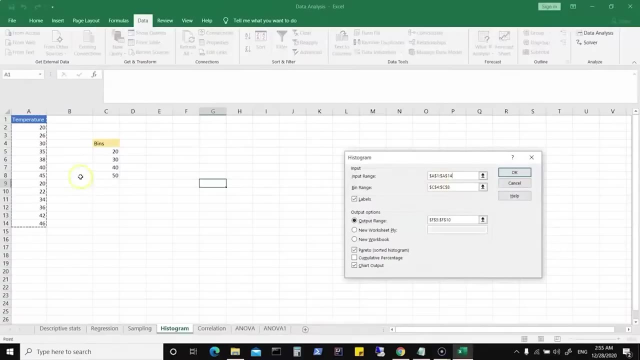 So we have already added the add-in, which is data analysis, earlier, So we can just use the same thing again Here we would want to create a histogram. So let's say, okay, Now I have already selected input range. So if you see, here my input range is temperature. 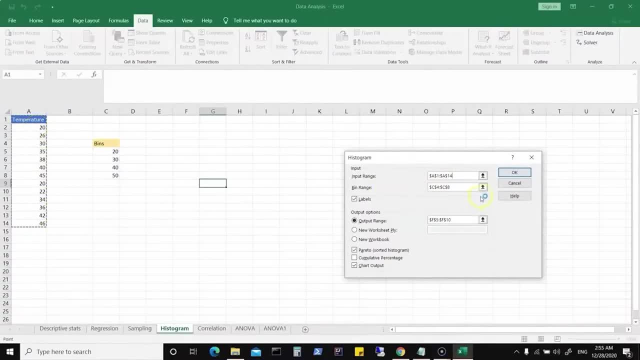 Which is also with the headings, And I have bin range, Which is basically the range of values. So, for example, I can select this And that's my bin range. I am selecting, or the option labels, Because I am using the first row. 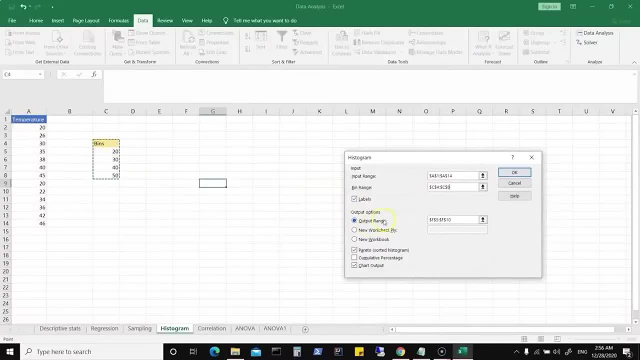 Which has the headings such as temperature and bins. Now we need to give an output range. So, for example, let's say I would want my data here And that becomes my output range. So you can have a sorted histogram Or basically a Pareto chart. 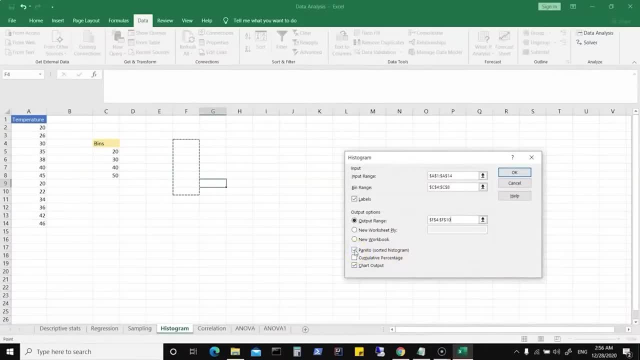 So, if that's what you are interested in- Looking at the frequencies for your different ranges- And here I am also selecting chart output, Because I would want to have a visual histogram Which gives us the frequency, And it's as simple as this. 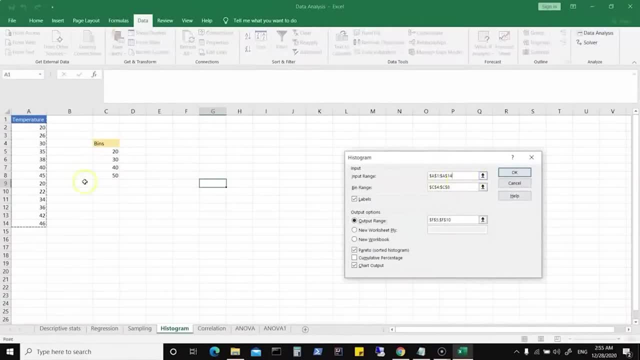 I have already selected input range. so if you see here my input range is temperature, which is also with the headings, and I have bin range, which is basically the range of values. so, for example, I can select this and that's my bin range. I am selecting the option labels because I am 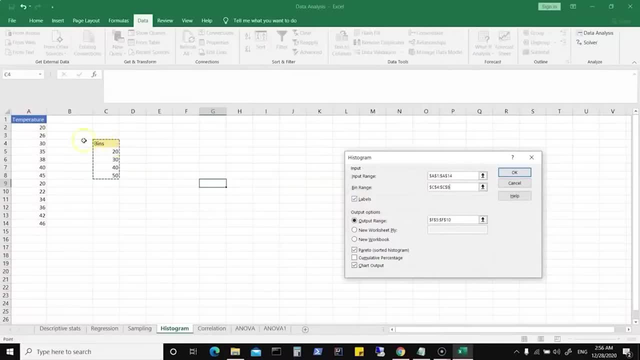 using the first row which has the heading such as temperature and bins. now we need to give an output range. so, for example, let's say I would want my data here and that becomes my output range. so you can have a sorted histogram or basically a Pareto chart. so 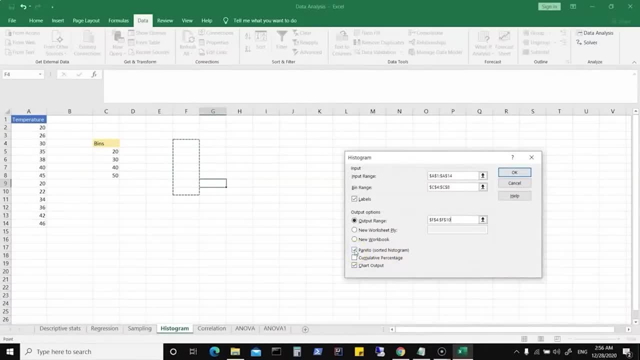 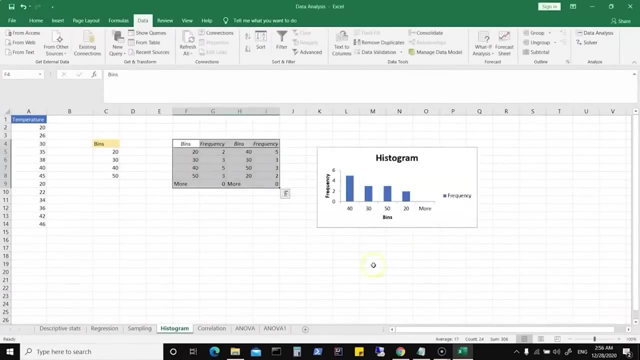 if that's what you are interested in: looking at the frequencies for your different ranges- and here I am also selecting chart output, because I would want to have a visual histogram which gives us the frequency. and it's as simple as this: just click on. ok, and now. 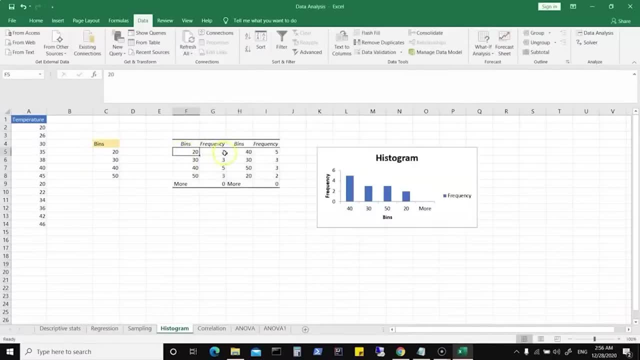 you get your bins. so it basically tells you frequency of values, which is basically 20, but that does not mean it is only talking about the values. 20, it is basically talking as a range of 0 to 20. so we have 0 to 20, that is 2, so we can. 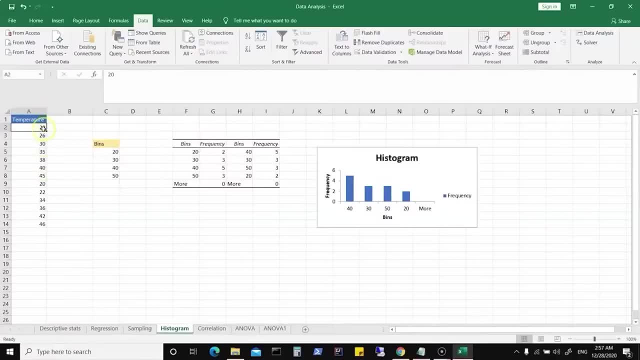 basically say there is 120 here, with the 20 being the maximum value, and then there is one more 20, so that's your 0 to 20. then you have 20 to 30, which shows 3 values. so might be in that case: 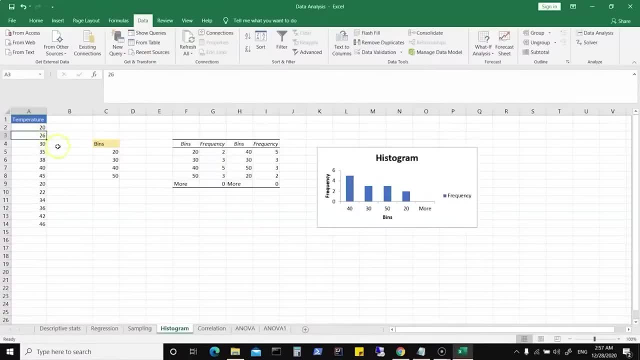 I can say 26 is one thing, then I can say 30, that's the second one, and then basically I can look at 22. so basically this one does not select 20 as the lower range, but it basically selects 30 as the higher range. 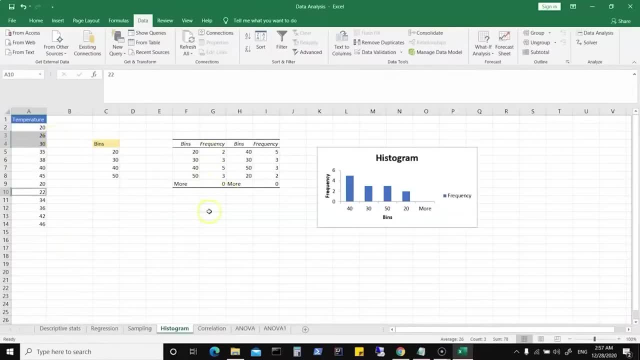 so I do see 22- 30. there are 3 entries. similarly, we can see values of 40 and 50 and since we have selected Pareto or sorted histogram that shows in a descending order what is the highest frequency of values within a particular range. 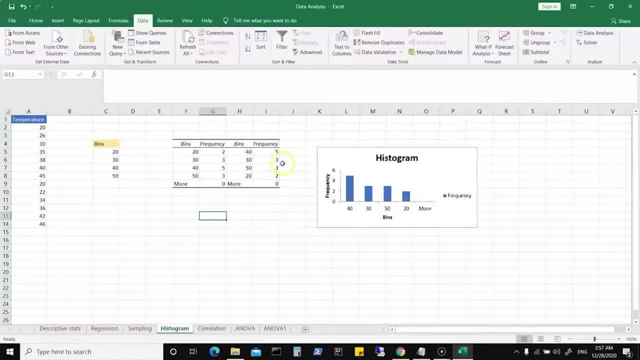 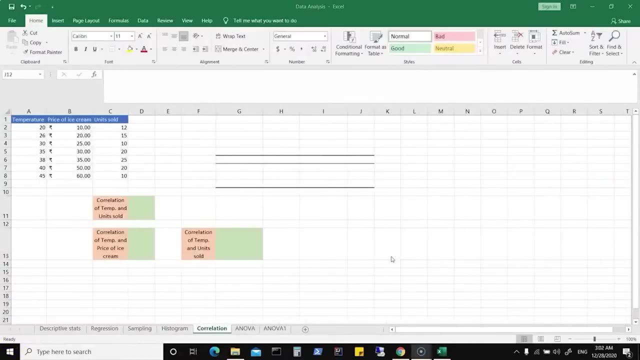 so that shows me highest frequency is 5, and then you have 3 and 3 and then 2. so this is how we can create a histogram and we can perform analysis on a single variable. now, as discussed earlier, as I said, sometimes we may be interested in. 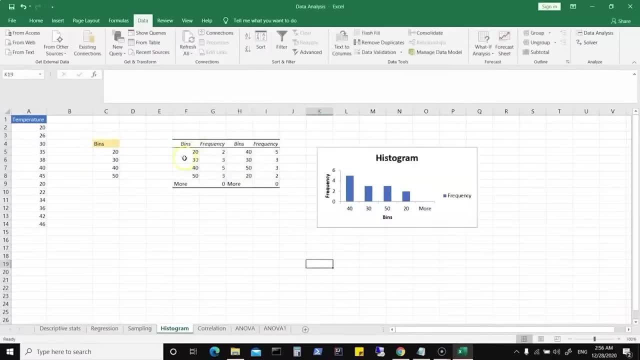 Just click on, okay, And now you get your bins. So it basically tells you frequency of values, Which is basically 20.. But that does not mean it is only talking about the values 20. It is basically talking as a range of values. 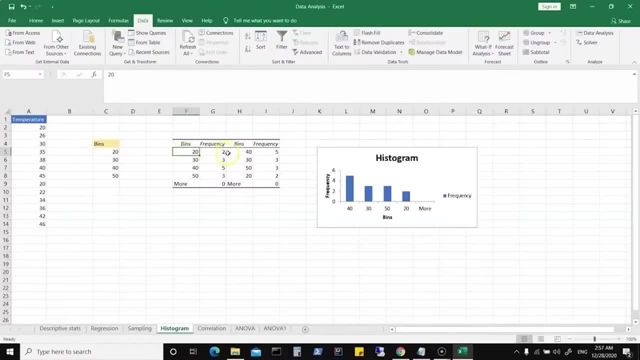 0 to 20.. So we have 0 to 20.. That is 2.. So we can basically say: there is one 20 here, With the 20 being the maximum value, And then there is one more 20.. So that's your 0 to 20.. 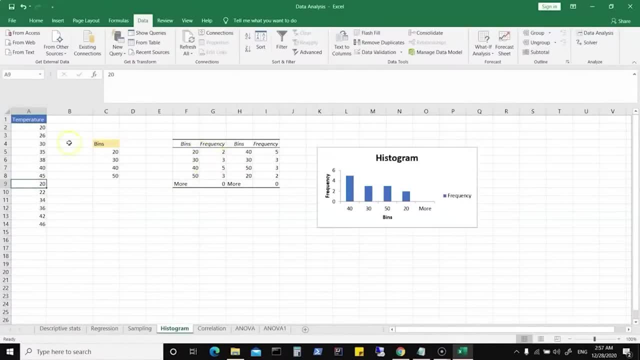 Then you have 20 to 30. Which shows three values. So might be. in that case I can say 26. Is one thing, Then I can say 30. That's the second one, And then basically I can look at 22.. 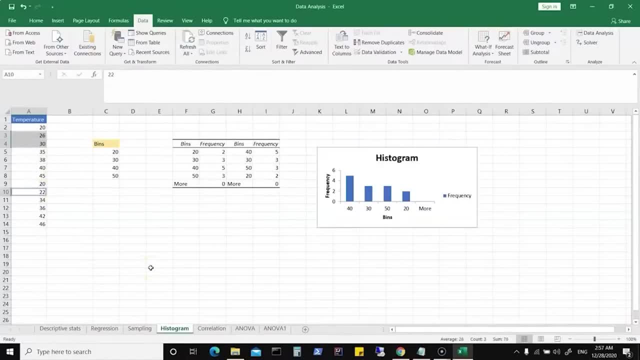 So basically, this one does not select 20 as the lower range, But it basically selects 30 as the higher range. So I do see 20 to 30.. There are three entries. Similarly, we can see values of 40 and 50.. 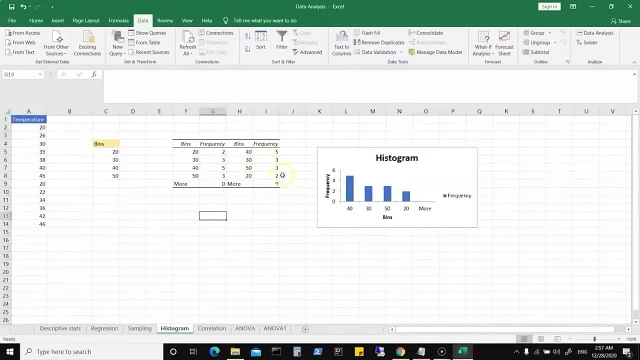 And since we have selected Pareto or sorted histogram, That shows in a descending order What is the highest frequency of values within a particular range, So that shows me highest frequency is 5.. And then you have 3 and 3 and then 2.. 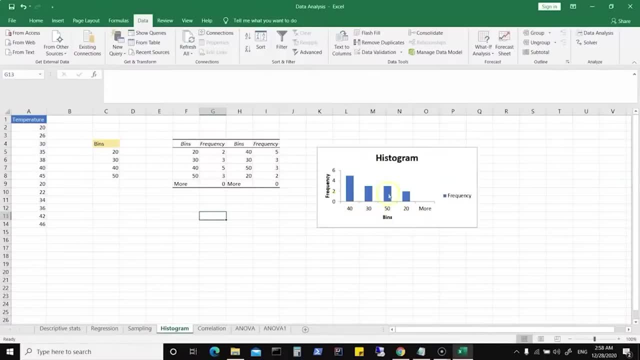 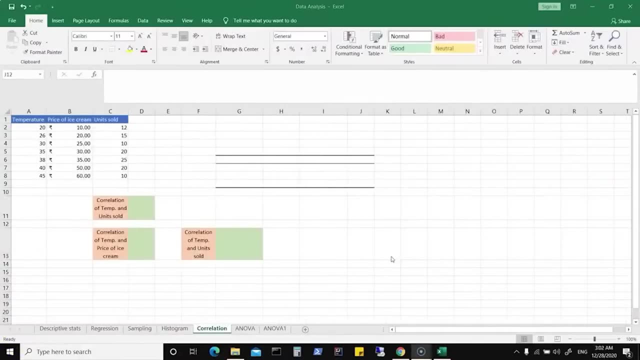 So this is how we can create a histogram And we can perform analysis on a single variable. Now, as discussed earlier, As I said, sometimes we may be interested in finding out the correlation between different variables, Such as, say, here we have temperature, price of ice cream and units sold. 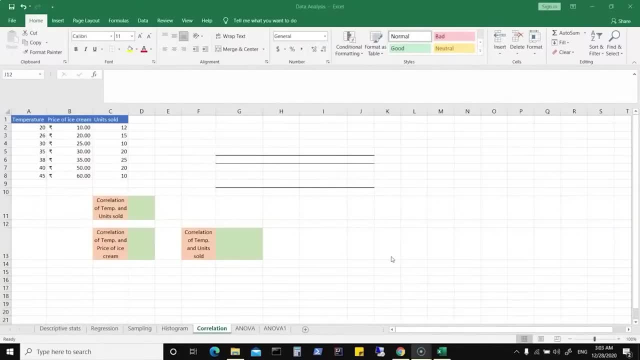 And we may want to find out The correlation between one variable to another variable. Or we would want to find out the relationship between variables. Are they linearly related, Are they positively related, Negatively related, And so on? And for that we can use the correlation of your data analysis. add in: 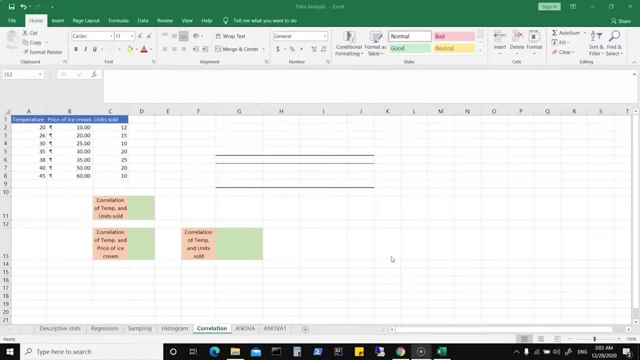 finding out the correlation between different variables, such as, say, here we have temperature, price of ice cream and units sold, and we may want to find out the correlation between one variable to another variable. or we would want to find out the relationship between variables. are they linearly related? 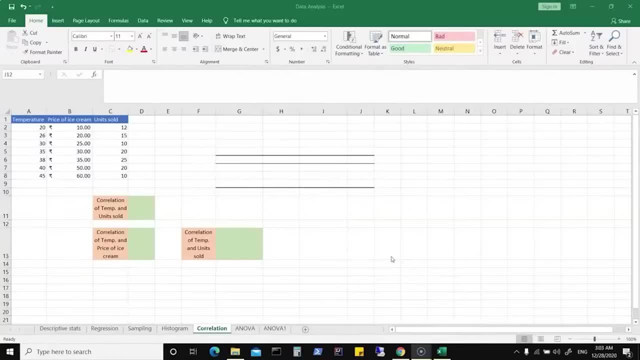 are they positively related, negatively related and so on, and for that we can use the correlation of your data analysis. add in so, for example, you want to find out correlation of temperature and units sold, and what we can do is we can find out that using a formula. 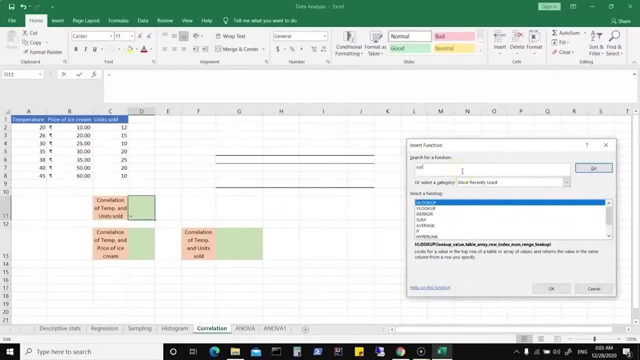 so, for example, if I search for something like co relation, and let's search. so there is a function called correlation which we can use, and we can use this to calculate the correlation of temperature and units sold. so, for example, let's select this and that's the function. so it says: 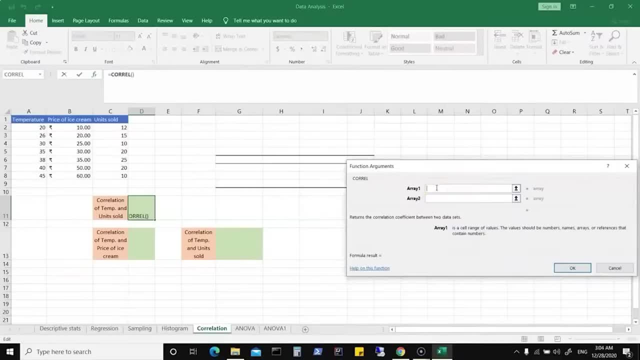 give me a first array and a second array. so we are interested in finding out correlation of temperature and units sold, so let's select the range of values for temperature. and then I am interested in finding out the correlation of temperature and units sold, so let's select. 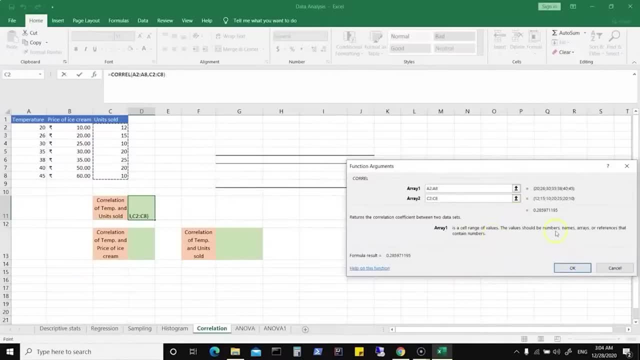 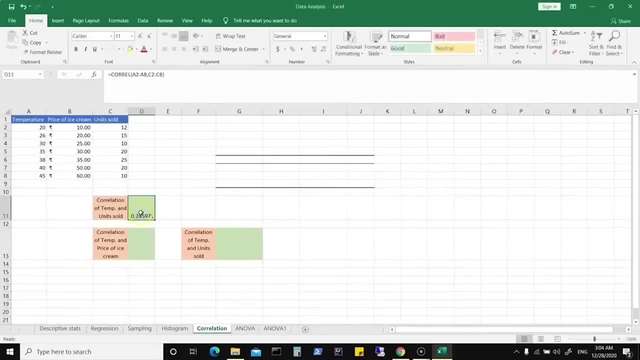 this and that basically gives me a range of values. it gives me the correlation value, which is 0.2859. say, ok, and that's your value. so similarly, we can do it for temperature and price ice cream. so let's go for correlation. so that's the function we are interested in. 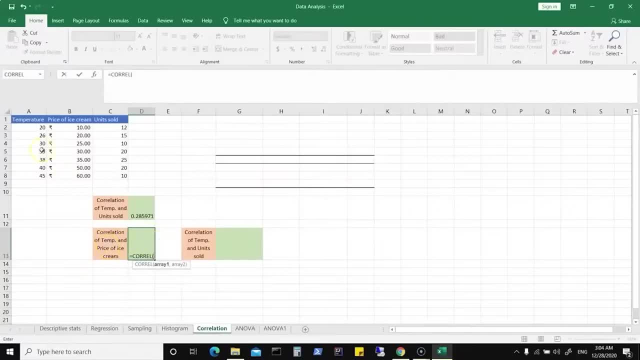 you need to give a range of values. so here we are interested in temperature and price of ice cream. so let's select temperature and then the second array or list of values is price of ice cream. let's select that, let's close our bracket and here we have. 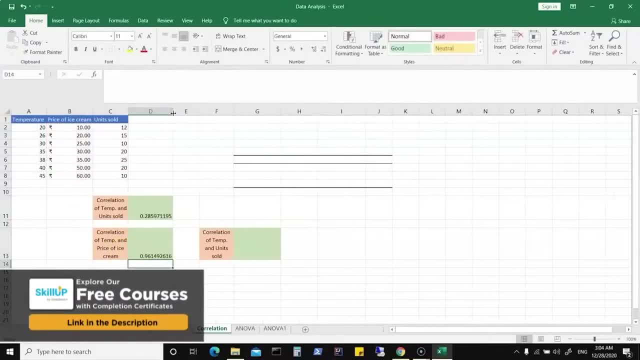 the correlation value of temperature and the price of ice cream. similarly, you may be interested in finding out temperature and units sold, like what we have done earlier. so we can do the same thing based on function. so this is same as correlation of temperature and units sold, so I can get rid of this one. 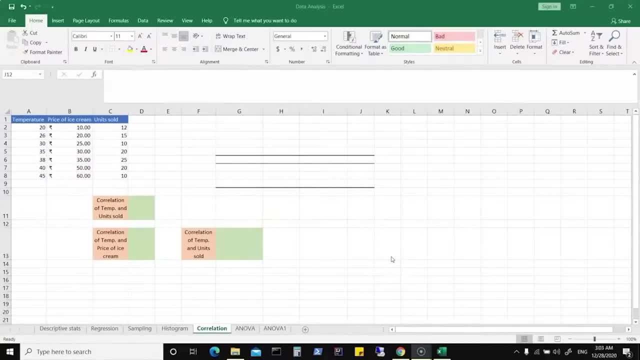 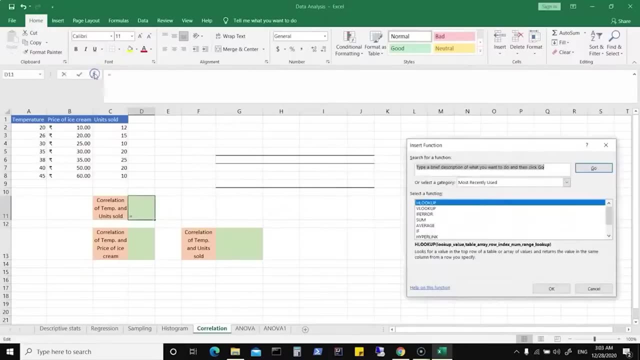 So, for example, you want to find out correlation of temperature and units sold, And what we can do is We can find out that Using a formula. So, for example, if I search for something like Correlation And let's search, So there is a function called correlation which we can use. 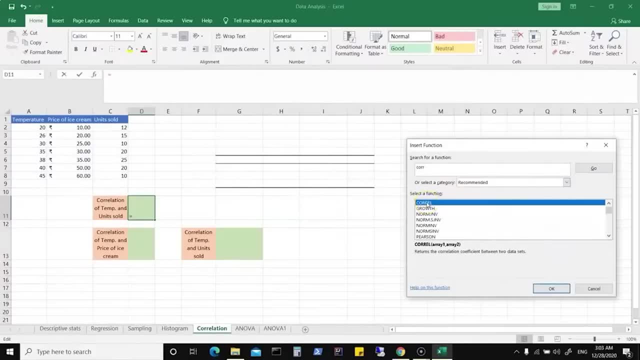 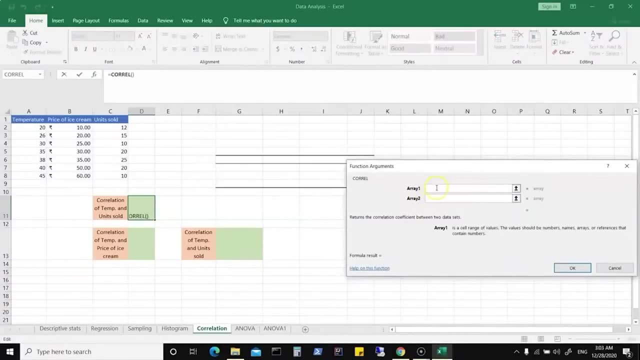 And we can use this to calculate the correlation of temperature and units sold. So, for example, let's select this And that's the function. So it says: give me a first array and a second array. So we are interested in finding out correlation of temperature and units sold. 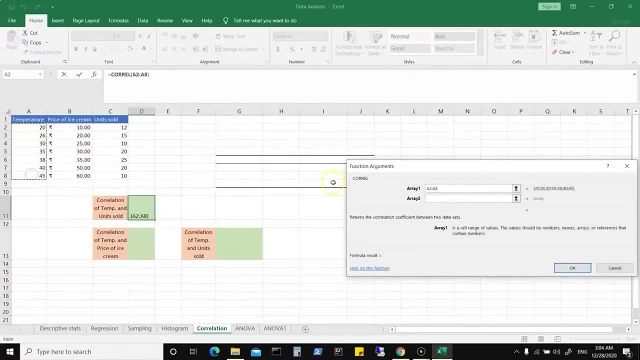 So let's select The range of values for temperature. And then I am interested in finding out the correlation of temperature and units sold. So let's select this And that basically gives me a range of values. It gives me the correlation value, which is 0.2859.. 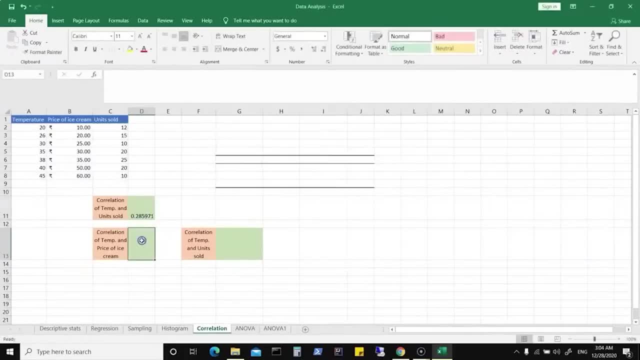 Say OK, And that's your value. So similarly, We can do it for temperature and price ice cream. So let's go for Correlation. So that's the function we are interested in. You need to give a range of values. 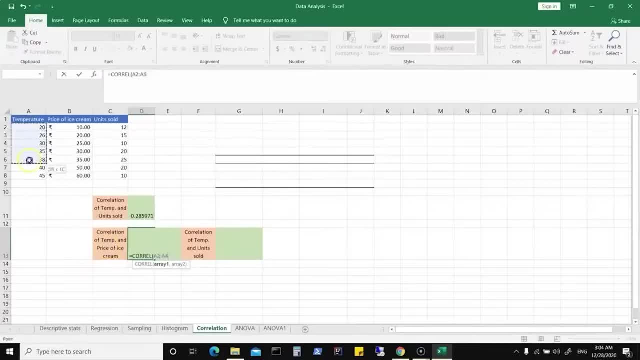 So here we are interested in temperature and price of ice cream. So let's select temperature, And then the second array or list of values is price of ice cream. Let's select that, Let's close our bracket And here we have the correlation value. 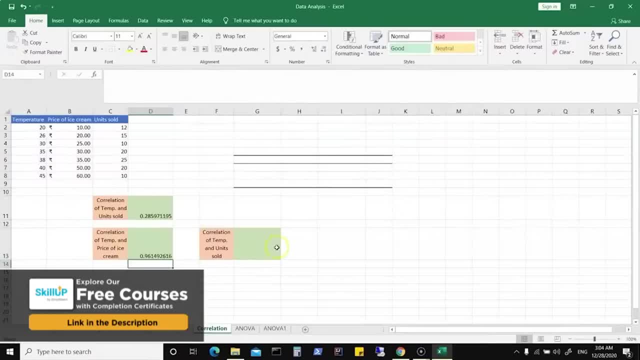 Of temperature And the price of ice cream. Similarly, You may be interested in finding out Temperature and units sold, Like what we have done earlier. So we can do the same thing Based on function. So this is same as Correlation of temperature and units sold. 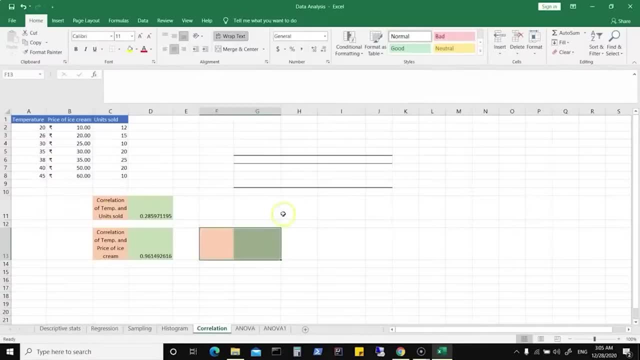 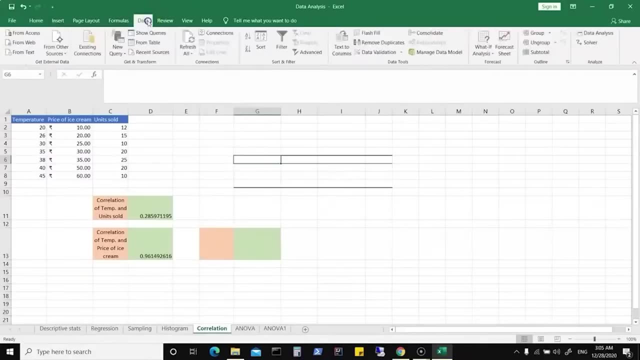 So I can get rid of this one. Now, how do I do it? using the data analysis add in. So, for that, What we need is We need to go into data, We need to click on data analysis And here you have the option called correlation. 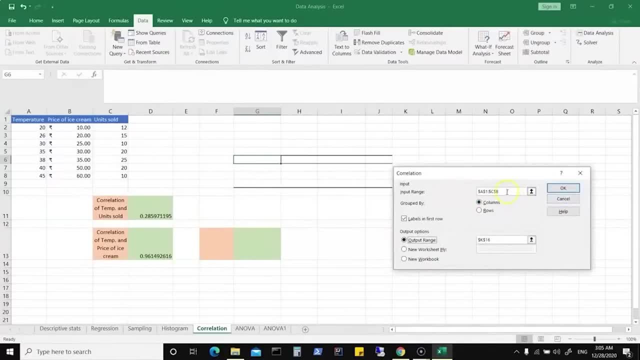 Let's select this Now. that basically needs an input range, So we need The range Now. I might be interested in finding out the correlation between temperature and price of ice cream and units sold. So I've selected all the columns here. We will say group by columns. 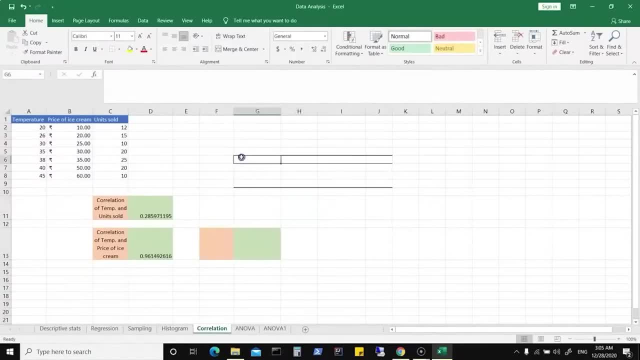 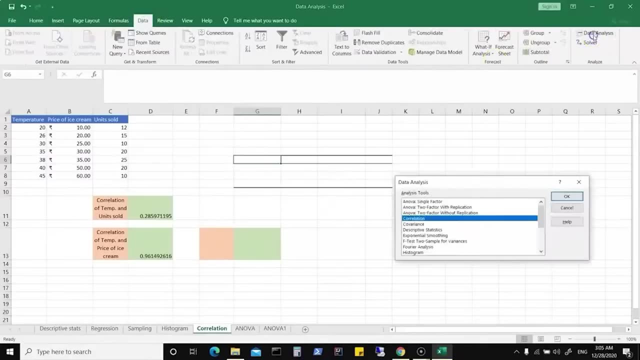 now, how do I do it? using the data analysis add in. so for that, what we need is we need to go into data, we need to click on data analysis and here you have the option called correlation. let's select this. now that basically needs an input range, so we need 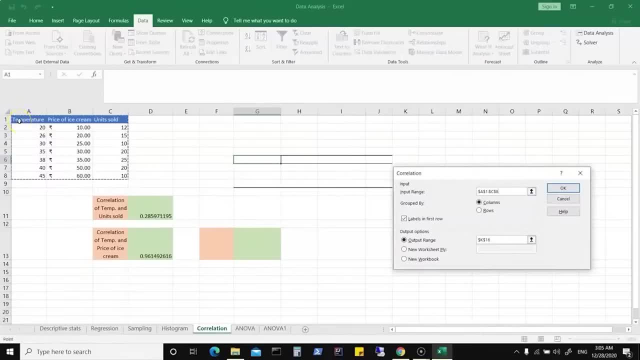 the range. now I might be interested in finding out the correlation between temperature and price of ice cream and units sold. so I have selected all the columns here. we will say group by columns. obviously we need to select labels in first row because that is basically taking care of the first row is heading. 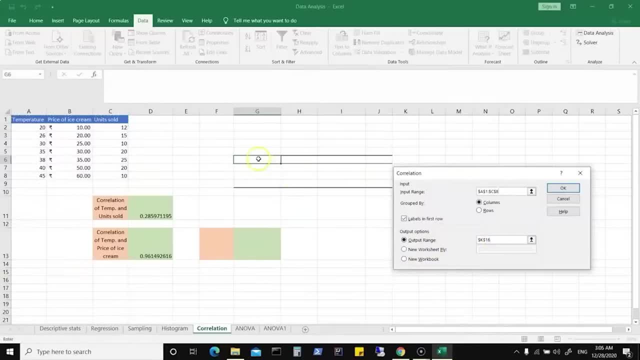 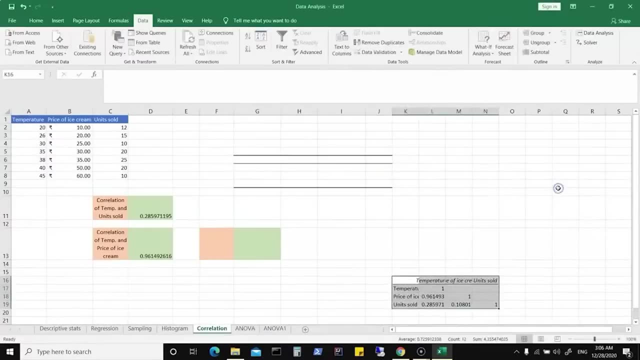 now output range. you can just give one simple cell and that's where your data will start from, or you can give a new workbook, so click on ok and that basically gives your. that basically gives your correlation of your different variables and what are the values and we can check these values. 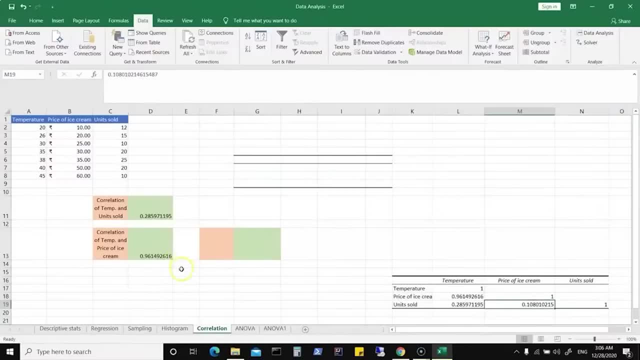 based on the values, what we have here. so we have basically temperature and price of ice cream and that basically shows me 0.96149. you have temperature and units sold, so you have 0.2859. now you can also look at units sold and say, for example, price of. 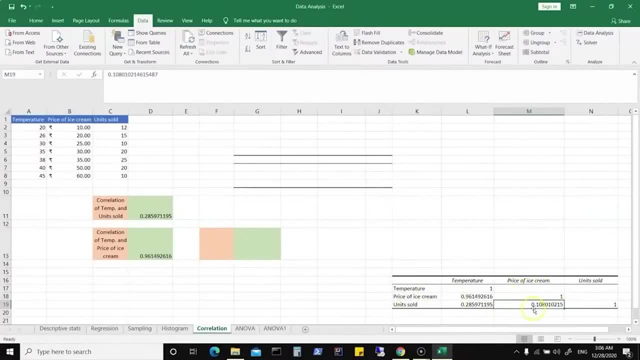 ice cream. you can look at these particular values. so if I would be interested in finding out what is the relationship between these variables, I can easily find using correlation, so I could be basically writing in a formula here and selecting what are the cells. so here we were selecting. 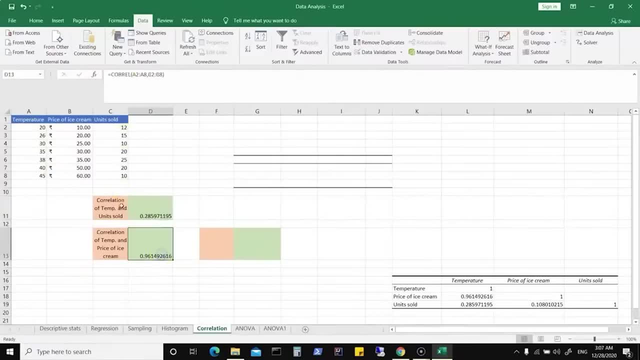 A2 and C. here we were selecting A and B. now might be. I am interested in price of ice cream and units sold, and if that's what I am interested in, then I will give a range of B2 to B8, C2 to C8 and similarly. 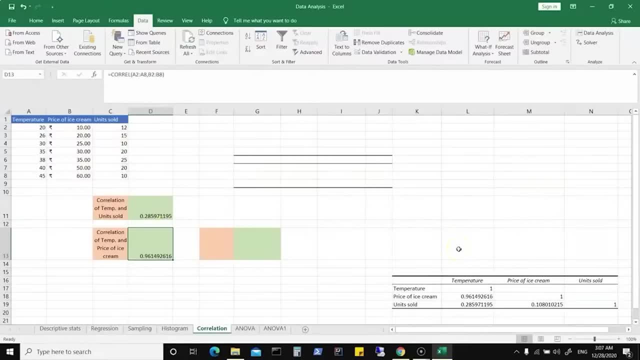 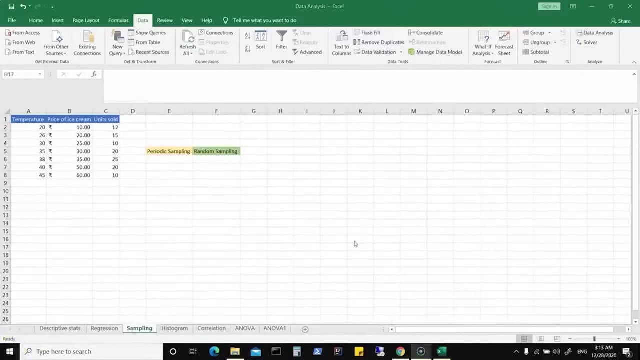 you can get your analysis or correlation values. so it's very simple in excel and you can use either the data analysis tab and get your correlation, or you can use formulas and do that. now. one more important part of data analysis is doing your sampling. now. sampling could be periodic. 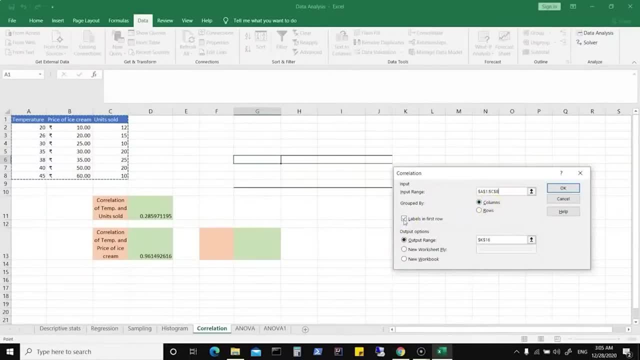 Obviously, we need to select labels in first row, Because that is basically taking care of the first row as heading. Now output range. You can just give one Simple cell. That's where your data will start from, Or you can give a new workbook. 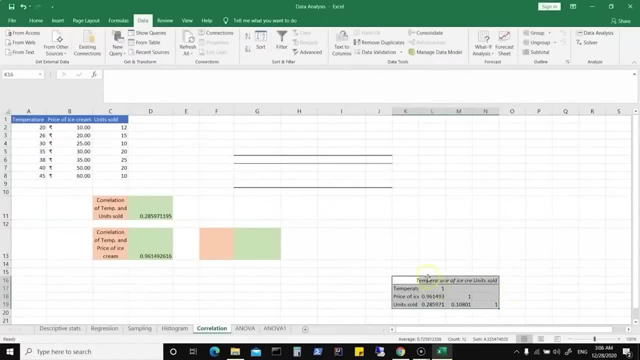 So click on OK And that basically gives your, That basically gives your Correlation of your different variables And what are the values, and we can Check these values Based on the values, what we have here. So we have basically Temperature. 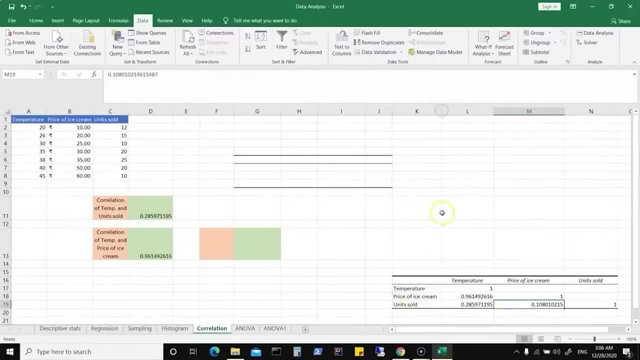 And price of ice cream. And that basically shows Me point nine, six, one, four, nine. You have temperature and units sold. So you have point two, eight, five, nine. Now you can also look at units sold And say, for example, price of ice cream. 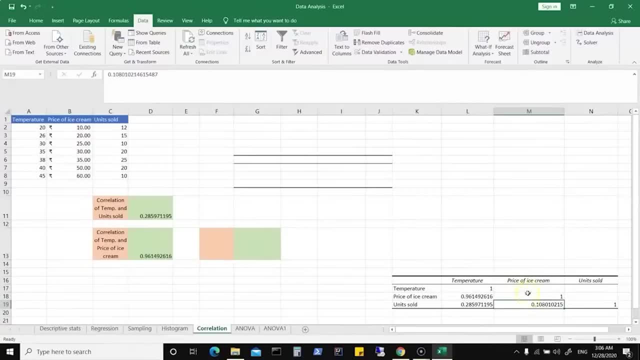 You can look at These particular values. So if I would be interested in finding out What is the relationship between these variables I can easily find using correlation, So I could be Basically writing in a formula here And selecting what are the sales. 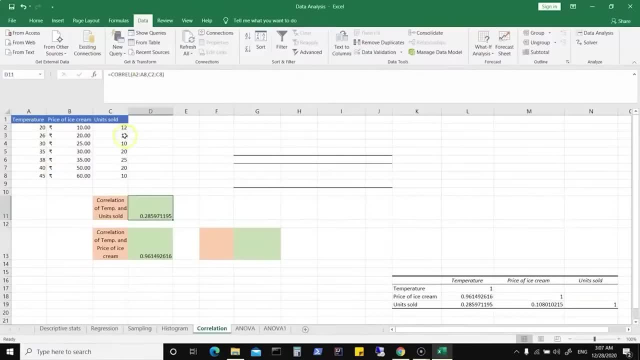 So here We were selecting eight, two And C. Here We were selecting A and B. Now might be I'm interested in price of ice cream And units sold, And if that's what I'm interested in, Then I will give. 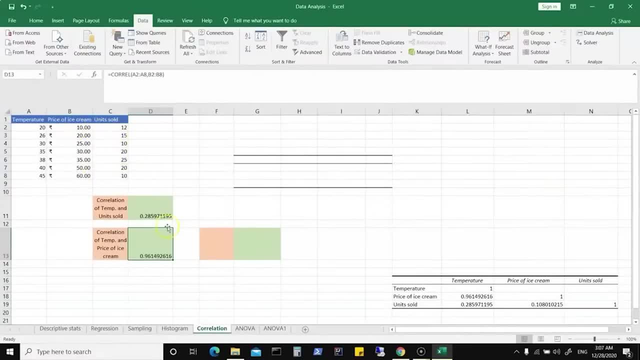 A range of B2. To B8, C2 to C8.. And similarly You can get Your analysis or correlation Values. So it's very simple in Excel And you can use Either the data analysis tab And get your correlation. 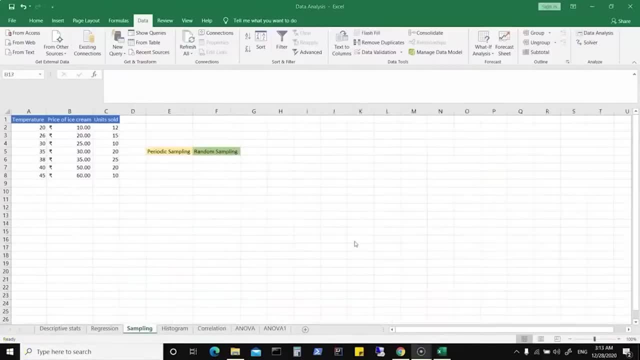 Or you can use formulas And do that. Now. one more important part of data analysis Is doing your sampling. Now sampling could be periodic sampling Or random sampling. So sometimes you may want to look at a variable And you may want to. 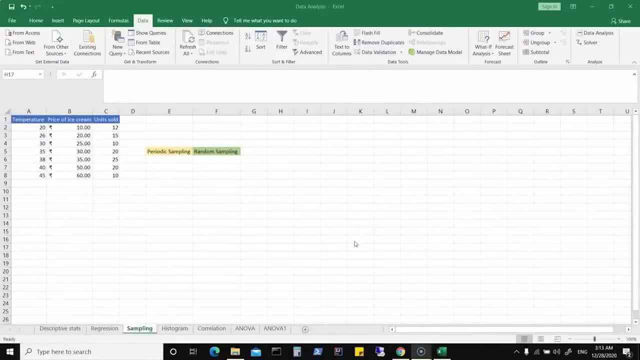 sampling or random sampling. so sometimes you may want to look at a variable and you may want to get some values based on periodic data. that means might be. I am interested in range of values. I am interested in seeing a sample of values for a particular period, which could be. 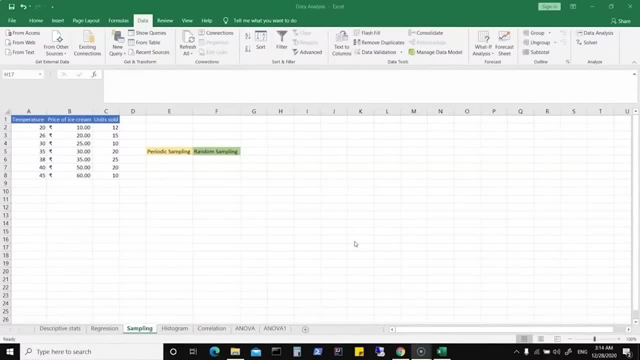 basically a range of values or you could just do a random sampling. so, for example, if I go for periodic sampling, so out of these values which I see here might be, I want to see, say, periodic sampling. that is a frequency of two values, how many times we? 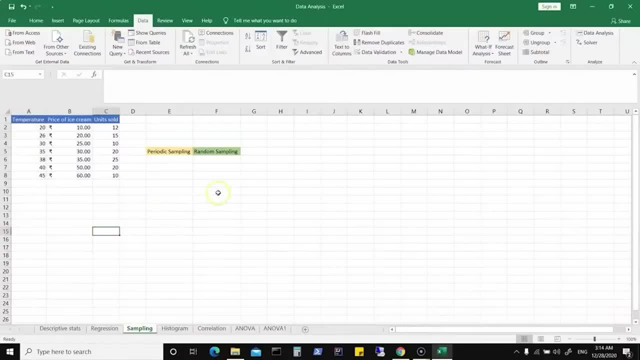 have these values occurring here, or I would go for random sampling. so basically randomly, I would want to pick up, say, three temperature values. now how do I do it? so, for example, here I have seven values. now if I go for periodic sampling, the sample or periodic sample- 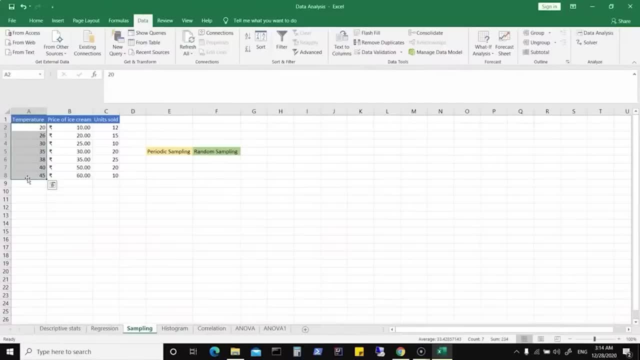 value which I need to give has to be lesser than the total input values. so, for example, we can do this, let's go in here and let's go for data analysis. so we can go for sampling here, click on ok, and that needs a range of values. so we 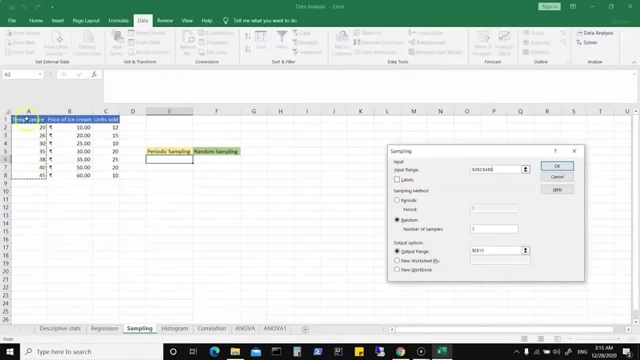 will select A2 to A8. now I could have selected all the values for this one temperature and in that case I can give labels, which is going to take care of the first row. now, here we can go for number of samples which we are interested in or giving. 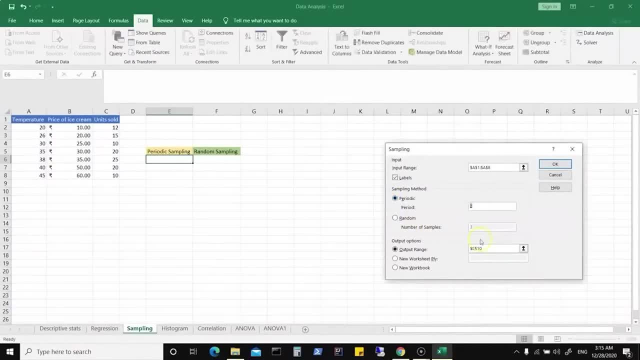 a period. so let's go for period and say, for example, I have seven values, so what if I select five? so for example, if I say five, that means I could just get one value. so basically, when I am saying five out of seven, so that's just giving me out of. 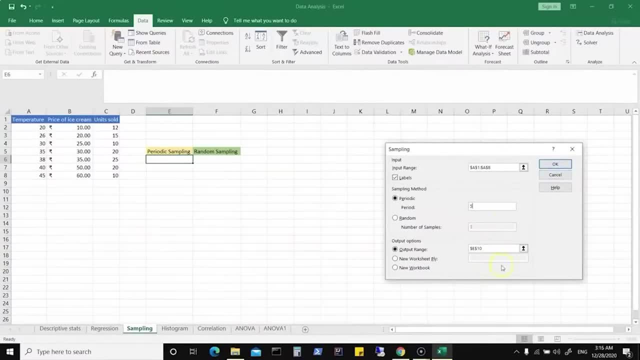 five. I want one value so I can then just give an output range. so here I can basically select this cell. I will say ok, and now you see, it just shows me one value. so out of the first range, that is, I have said five, it has given me the fifth value, that's. 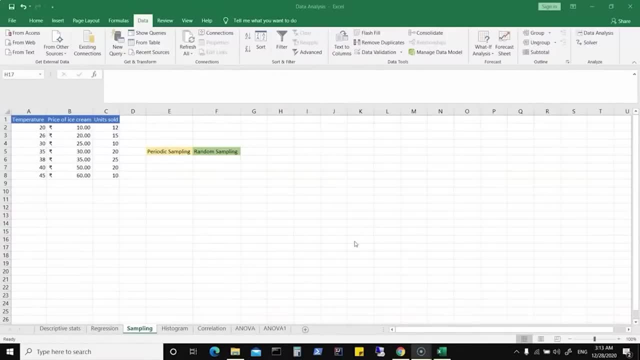 Get some values based on periodic data. That means Might be. I'm interested in Range of values. I'm Interested in seeing a sample of values for A particular period, Which could be basically A range of values Or you could just do a random sampling. 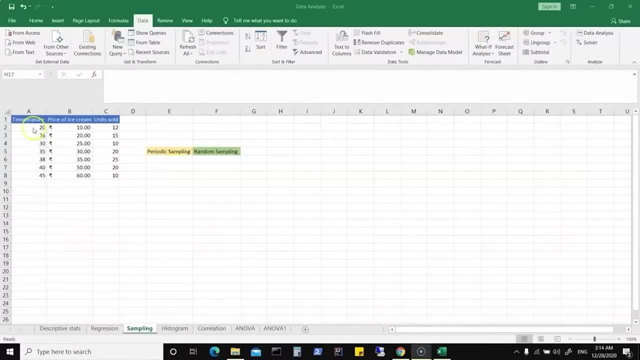 So, for example, If I go for periodic sampling, So out of these values Which I see here Might be, I want to see, Say, periodic sampling, That is A frequency of two values, How many times We have these values occurring here. 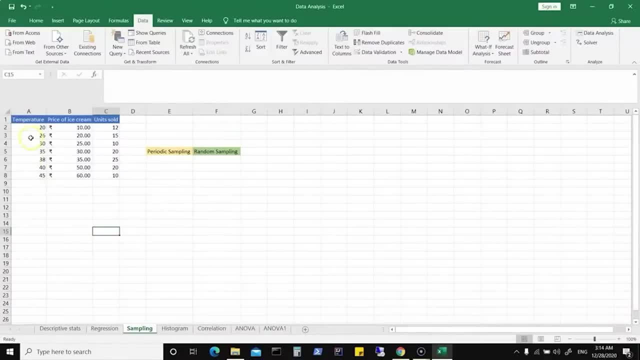 Or I would go for random sampling. So basically, randomly, I would want to pick up, Say, three temperature values. Now how do I do it? So for example, Here I have seven values. Now, if I go For periodic sampling, The sample, 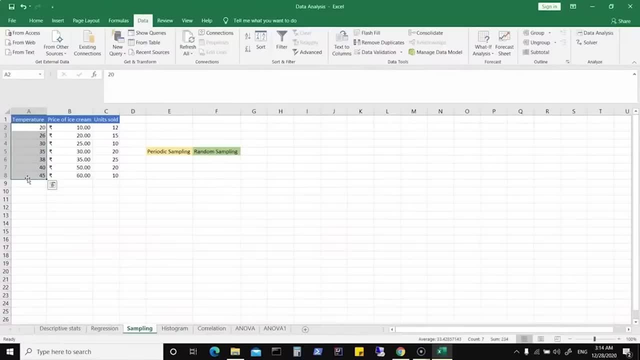 Or periodic sample value Which I need to give Has to be Lesser than The total Input values. So, for example, We can do this, Let's go in here. And let's go for data analysis, So we can go for sampling here. 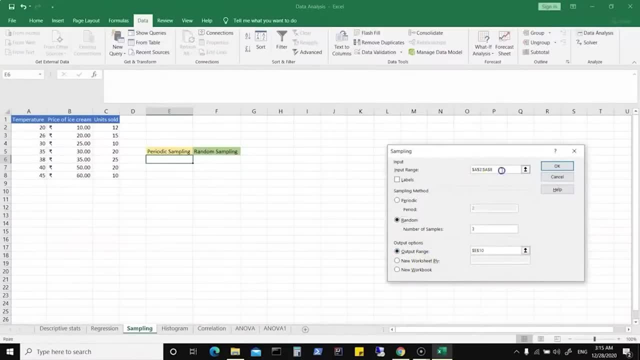 Click on OK, And that needs a range of values, So we will select A2 to A8.. Now I could have selected All the values For this one Temperature, And in that case I can give labels. Which is going to take care of the first. 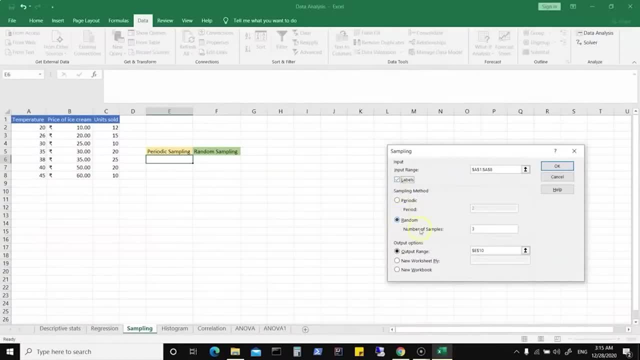 Row. And Now here We can go for Number of samples Which we are interested in Or Giving a period. So let's go for period And say, for example, I have seven values, So what if I select? 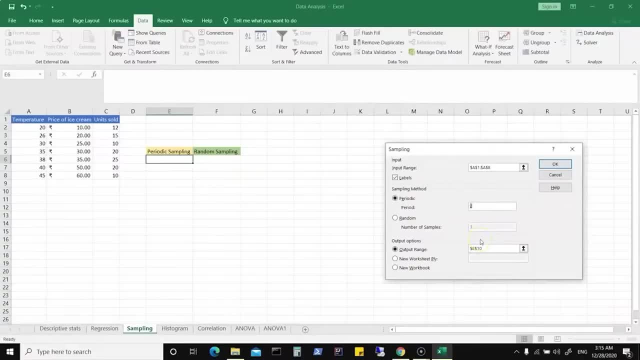 Five. So, for example, If I say five, That means I could just Get One value. So, Basically, When I'm saying Five Out of seven, So that's just giving me Out of five I want. 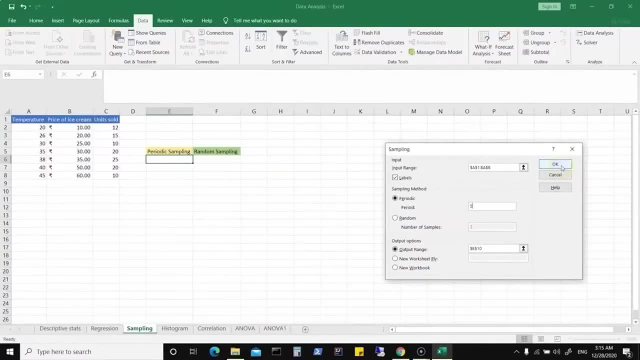 One value, So I could just Get One value, So I can Then just Give an output Range. So here I can Basically Select This cell. I'll say Okay, And now you see, It just shows me. 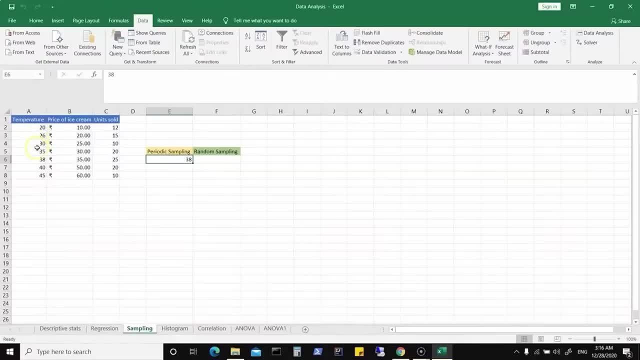 One value. So, Out of the first Range, That is, I've said, Five, It has given me The fifth Value, That's your Periodic Sampling. So, for example, We want More values Basically. 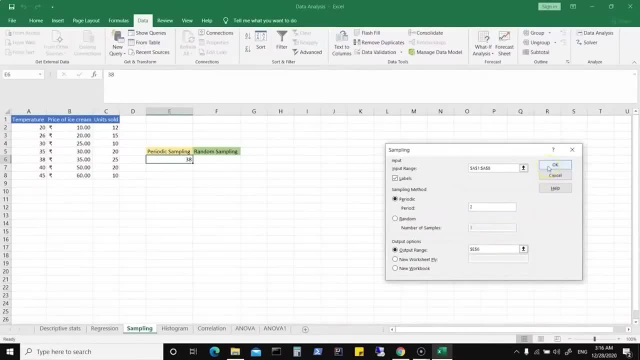 Gives me Every second Value. So I can Basically Say, For example, Two And say Okay, And then Say Okay. So that shows me Twenty Six, Then you have Thirty Five, Then you have. 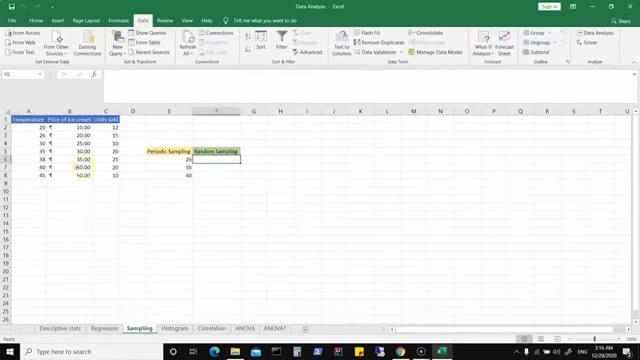 Forty And then Well, This one Does not have Any More Values. So Go For data Analysis, Go For sampling. I'll Go For Number Of Samples. How Many? 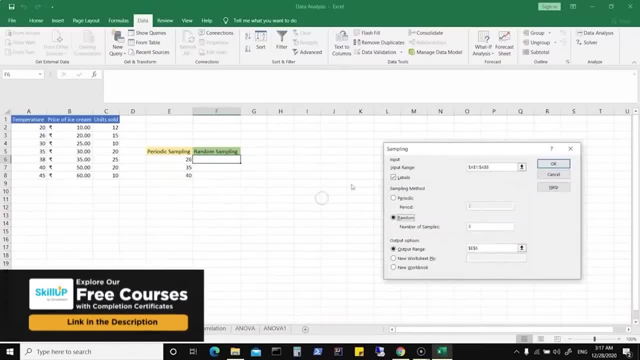 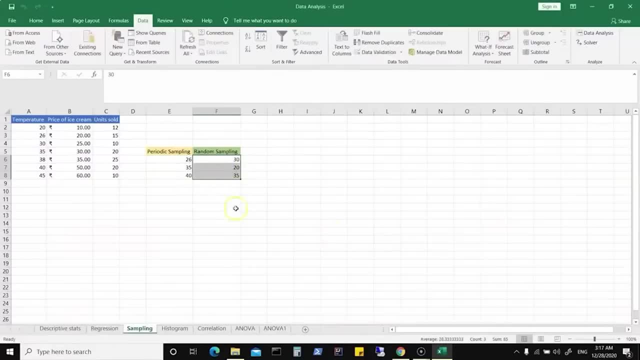 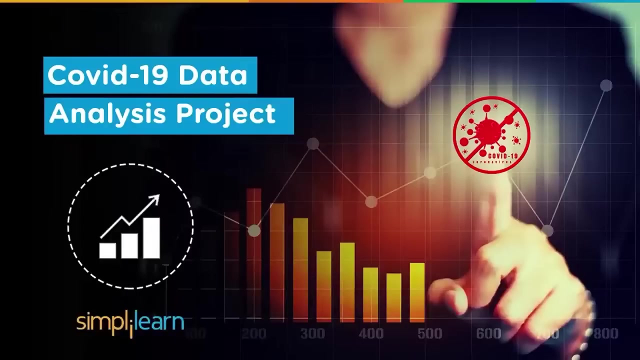 You Want. So For Example, Out Of Seven Values Randomly I Want Three Values And I Want To Do A Simple Sampling And We Can. 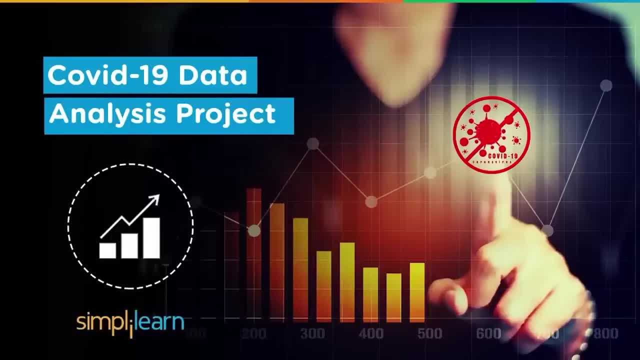 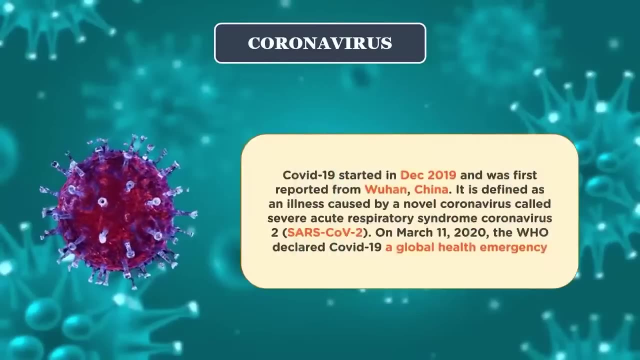 Choose Whether We Would Want To Go For People. Hello Everyone, And Welcome To This Interesting Video Tutorial By Simply One And Other, As You Think. 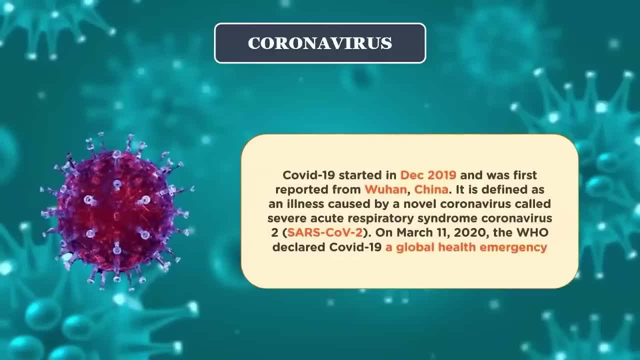 About Us And How You Can Save Your Life And Your Health And Your Life, And Your Life And Your Life And Your been. over 3.3 crore confirmed cases and nearly 4,41,000 deaths have been reported so far. 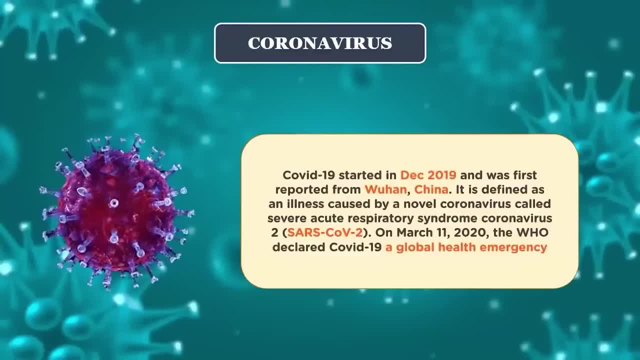 This data is according to official figures released by the Union Ministry of Health and Family Welfare. As the world tries to cope up with this deadly virus, we request all our viewers and their family members to follow all the necessary precautions to avoid getting infected. Quiz Time. 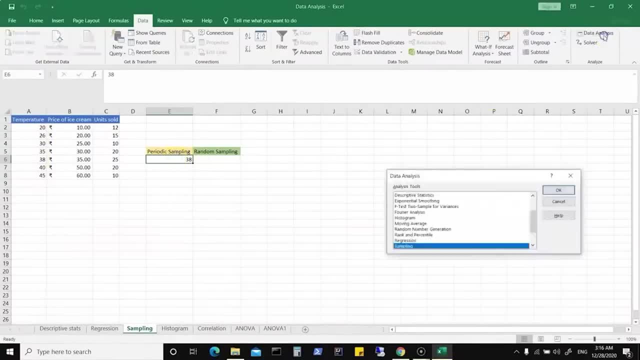 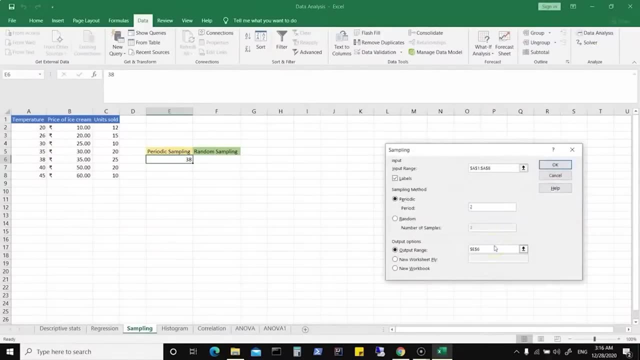 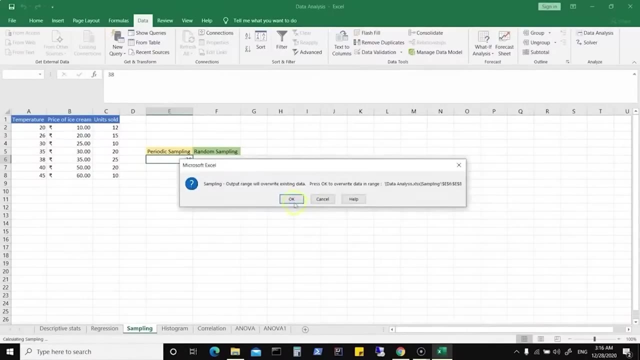 your periodic sampling. so, for example, we want more values, so let's reduce this period to might be two, which basically gives me every second value. so I can basically say, for example, two and say ok, and then say ok, so that shows me twenty six, then you have thirty five. 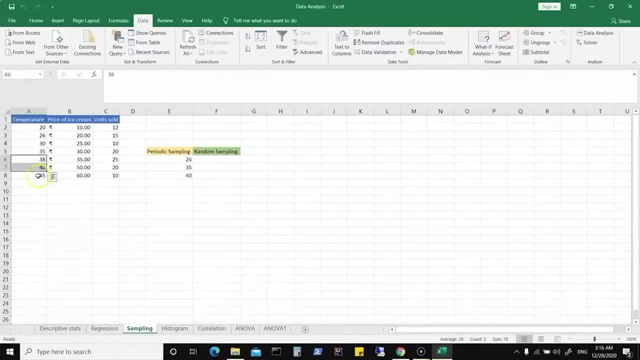 then you have forty and then, well, this one does not have any more values. so that's your period sampling. now, if you go for random sampling, that's basically randomly picking up values and you can choose how many values you want. so go for data analysis, go for sampling. 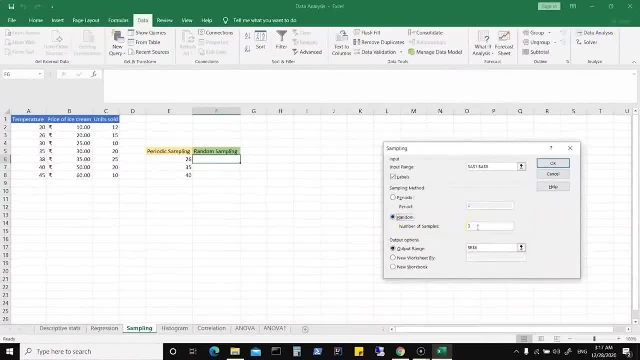 I'll go for number of samples, how many you want. so, for example, out of seven values randomly, I want three values and I can just give this, say ok, and then we will do a cancel because we need to change the range. so let's select this and say ok and that. 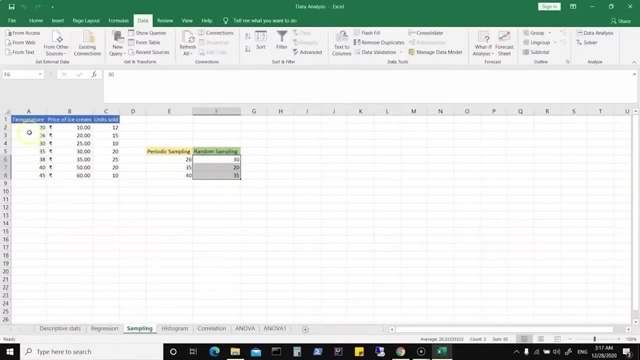 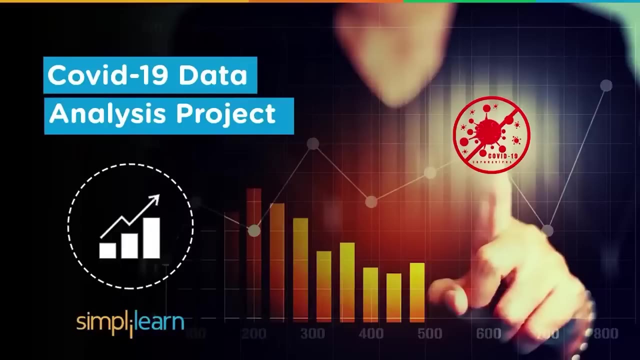 gives me random three values from this- values of temperature- so we can use excel to do a simple sampling and we can choose whether we would want to go for period. hello everyone and welcome to this interesting video tutorial. by simply learn. today we are going to perform two hands on projects on 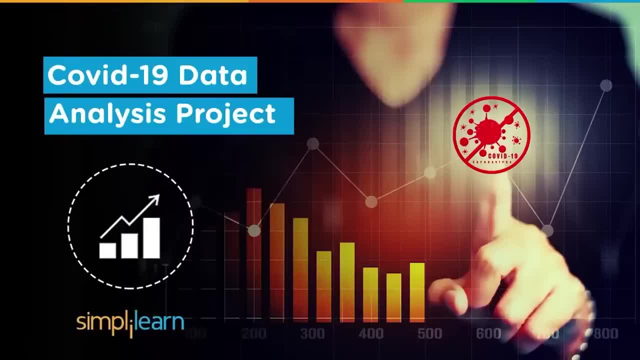 covid data analysis using python and tableau. this is going to be a really interesting and fun session where I'll be asking you a few generic quiz questions related to coronavirus. please make sure to answer them in the comment section of the video. we'll be happy to hear from you, covid. 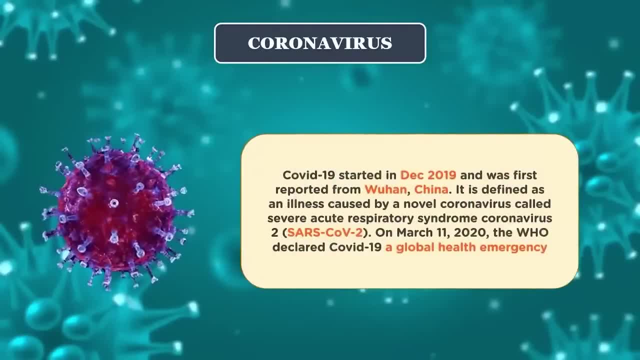 or coronavirus, is an ongoing global pandemic of coronavirus disease that emerged in 2019 and was first identified in Wuhan, China. it is defined as an illness caused by a novel coronavirus called severe acute respiratory syndrome coronavirus 2, commonly known as SARS-CoV-2. 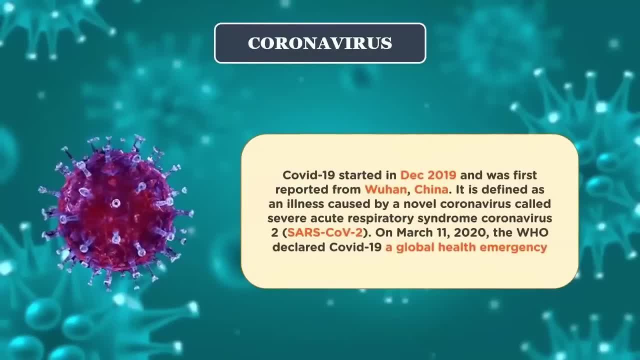 on March 11- 2020, the WHO declared covid-19 a global health emergency. the virus has so far infected over 22 crore people and killed more than 4.5 million innocents. in India, there have been over 3.3 crore confirmed cases and nearly 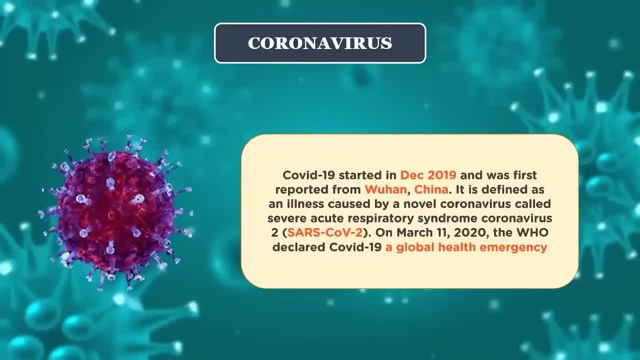 4,41,000 deaths have been reported so far. this data is according to official figures released by the union ministry of health and family welfare. as the world tries to cope up with this deadly virus, we request all our viewers and their family members to follow all the 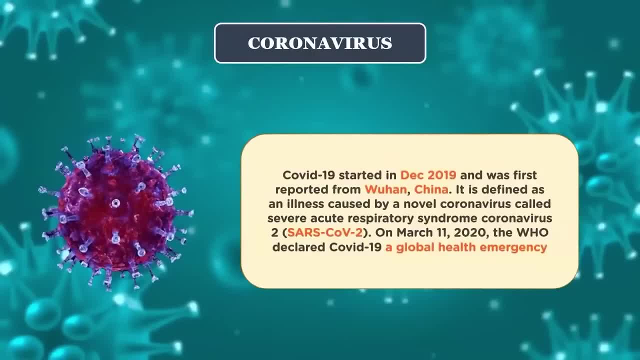 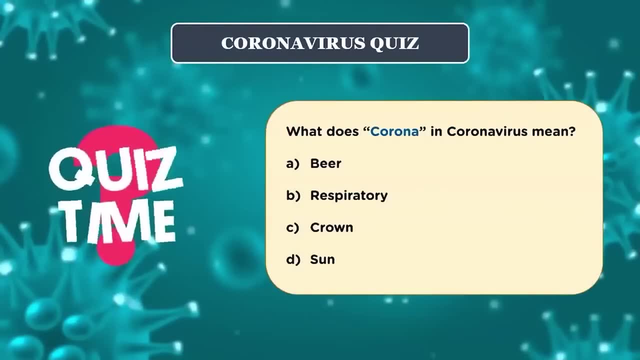 necessary precautions to avoid getting infected. quiz time now let's see our first quiz in this project. what does corona in coronavirus mean? here are the options: is it A beer, B respiratory, is it C crown or is it D sun? this is a very generic question. I am sure a lot of you may already. 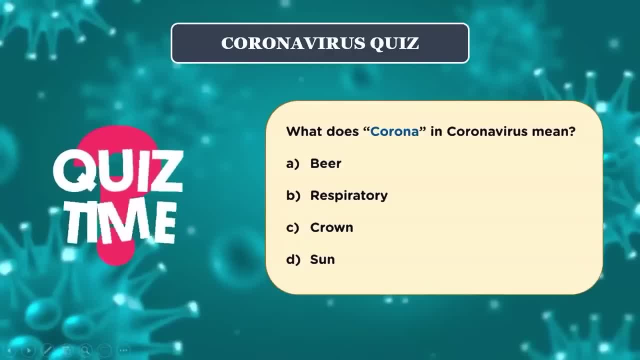 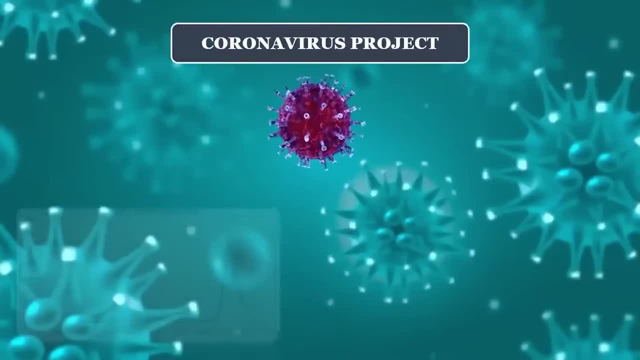 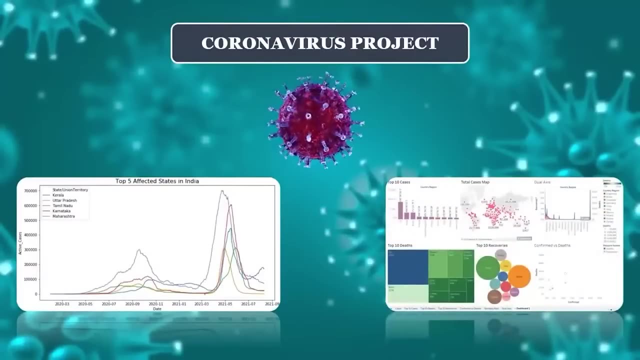 know some of you may not. please let us know your answers in the comment section of the video. we will be glad to hear from you now. in this video we will use three different covid-19 data sets and perform data analysis using python and tableau. the project. 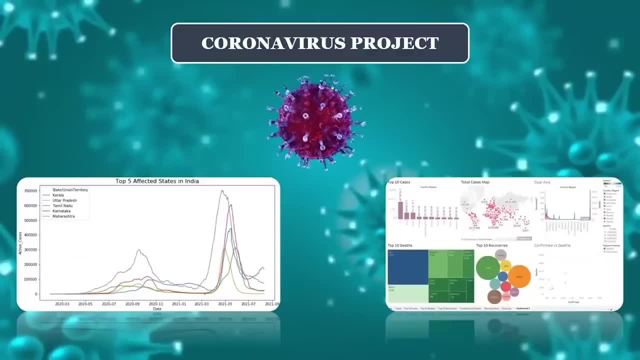 will give you hands-on experience working on real-world data sets and how you can use the different python libraries to analyze and visualize data and draw conclusions. you will learn how to create different plots in tableau and then make a dashboard from the visuals. the project will give you an idea about the impact. 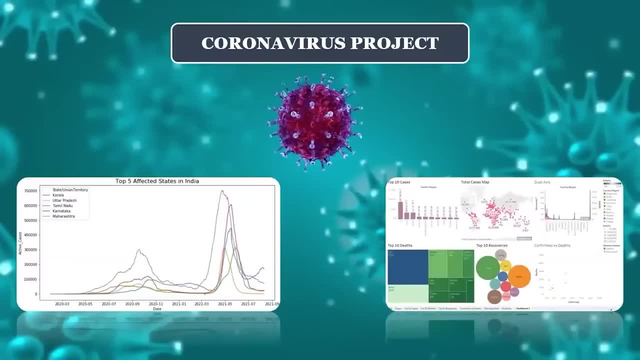 of coronavirus globally, in terms of confirmed cases, deaths reported, the number of recoveries, as well as active cases. we will also see how India has been affected since the pandemic started and dive into the different states and union territories to learn more about the covid-19 influence. 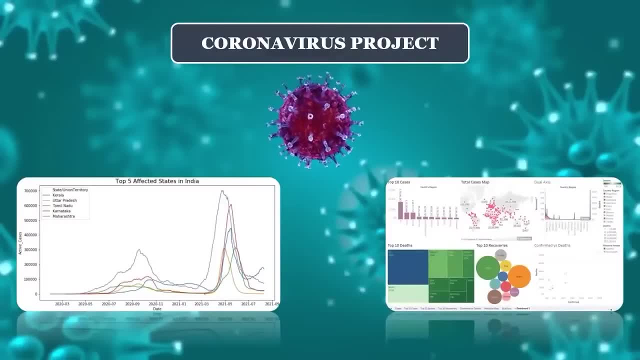 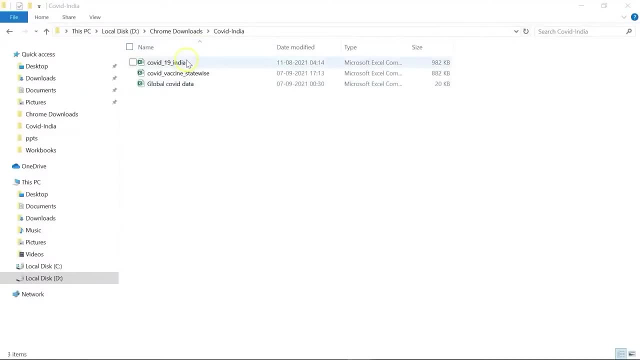 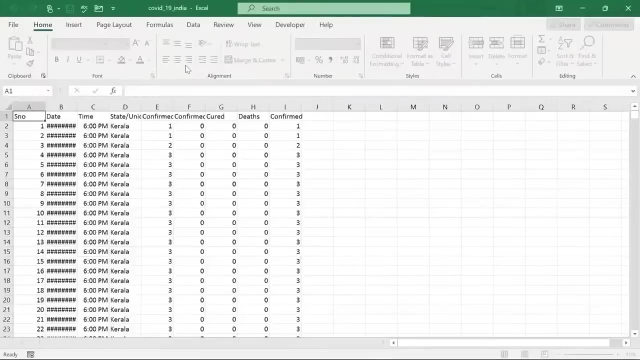 and the vaccination status. first, let me show you the two data sets that we will be using. so for our first project using python, we will be using the first two data sets: covid-19 India and covid vaccine statewide. let me open the two data sets. ok, so 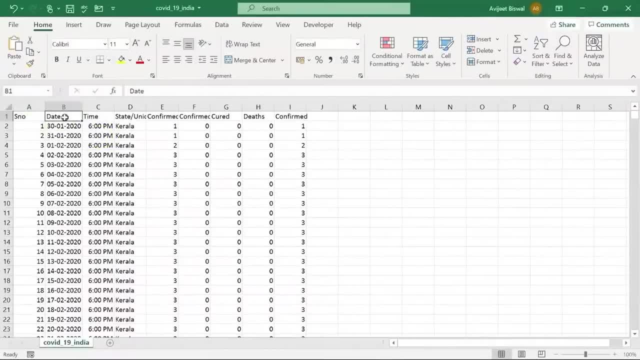 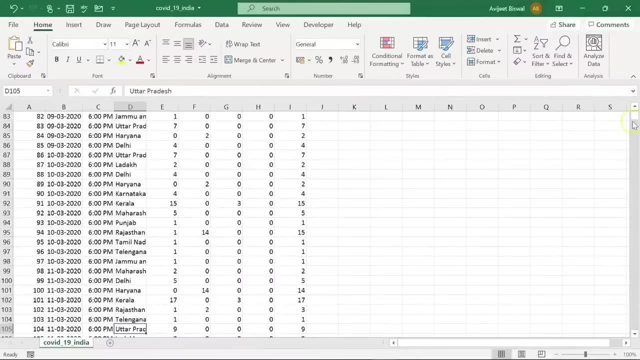 this is the first data set you can see. here we have the date, we have the time. then we have the different state names. scroll down you can see we have kerala, tamil nadu, delhi, hariana, rajasthan, ladakh, punjab, talangana and other states. then we 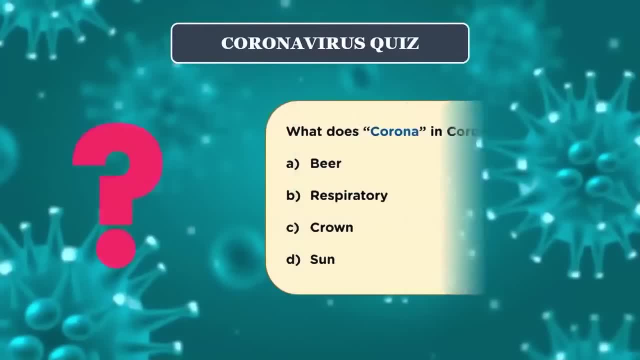 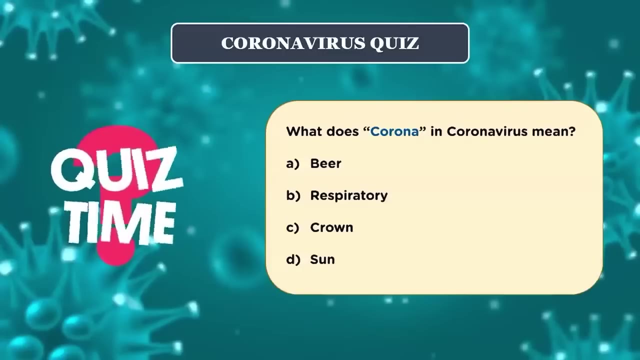 Now let's see our first quiz in this project: What does Corona in Coronavirus mean? Here are the options: Is it A Beer, B Respiratory, Is it C Crown or is it D Sun? This is a very generic question. I am sure a lot of you may already know, some of you. 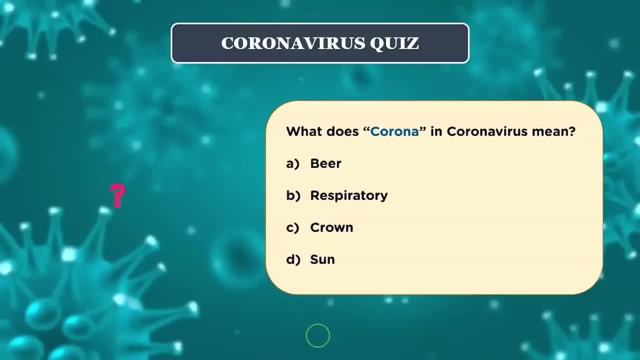 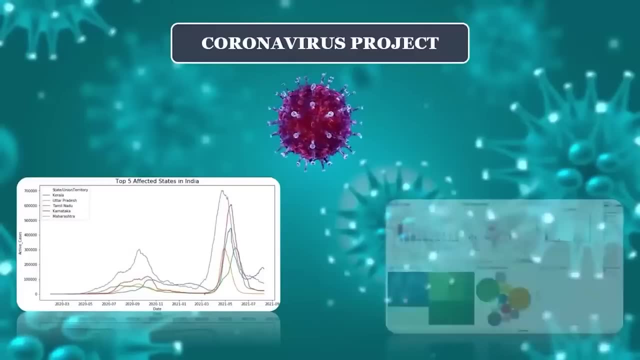 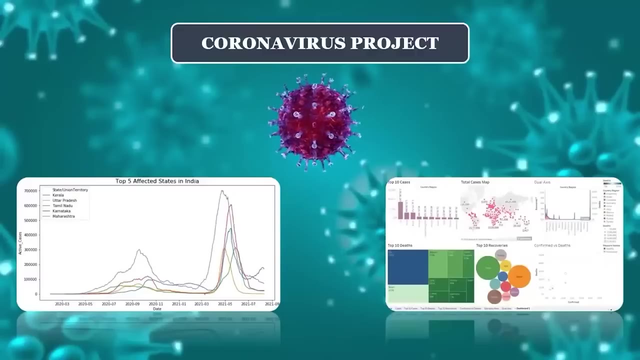 may not. Please let us know your answers in the comment section of the video. we will be glad to hear from you Now. in this video, we will use three different COVID-19 datasets and perform data analysis using them. The project will give you hands-on experience working on real-world datasets and how you 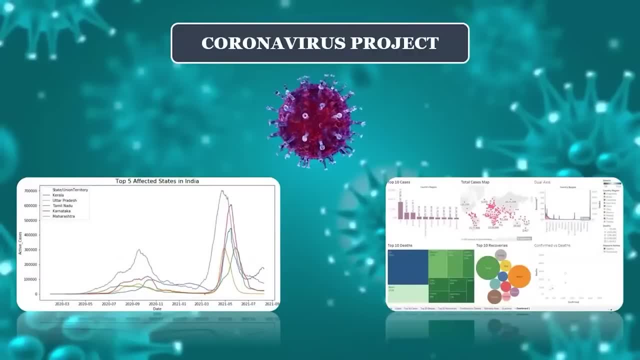 can use the different Python libraries to analyze and visualize data and draw conclusions. You will learn how to create different plots in Tableau and then make a dashboard from the visuals. The project will give you an idea about the impact of Coronavirus globally in terms of 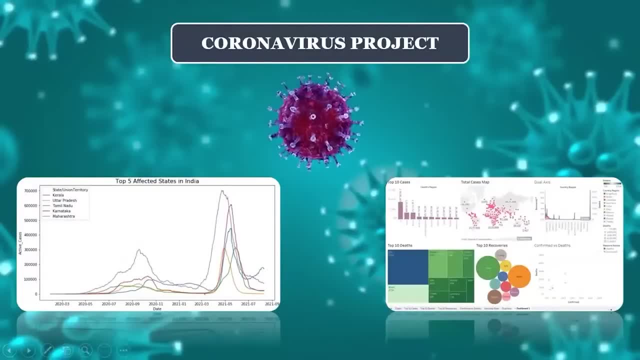 confirmed cases, deaths reported, the number of recoveries, as well as active cases. We will also see how it works. Let's see how India has been affected since the pandemic started and dive into the different states and union territories to learn more about the COVID-19 influence and the vaccination. 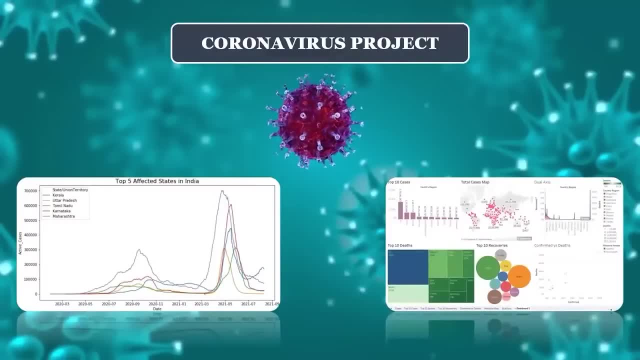 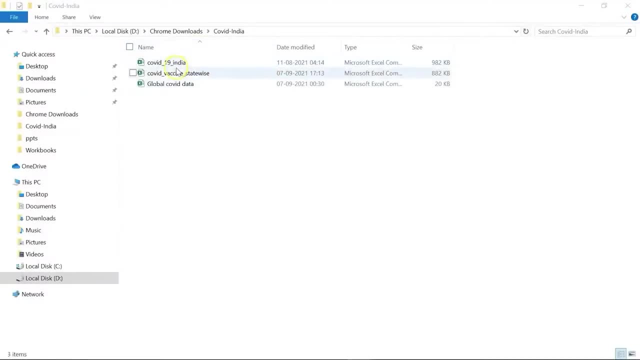 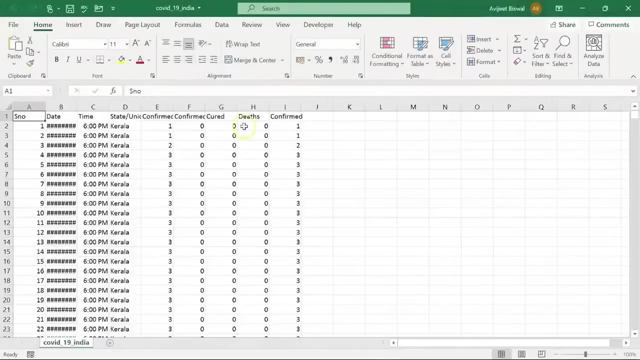 status. First, let me show you the two datasets that we will be using. So for our first project using Python, we will be using the first two datasets: COVID-19- India and COVID-19- Vaccine- state-wise. Let me open the two datasets. okay, so this is the first dataset you can see here. 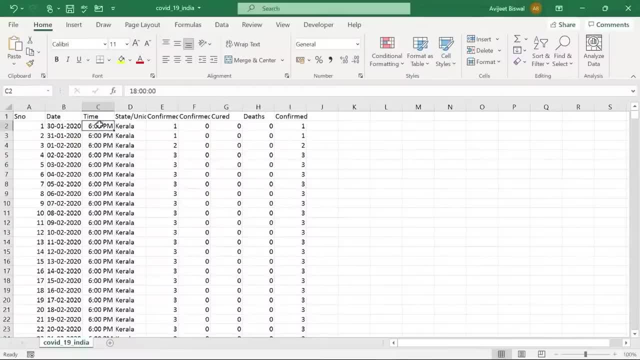 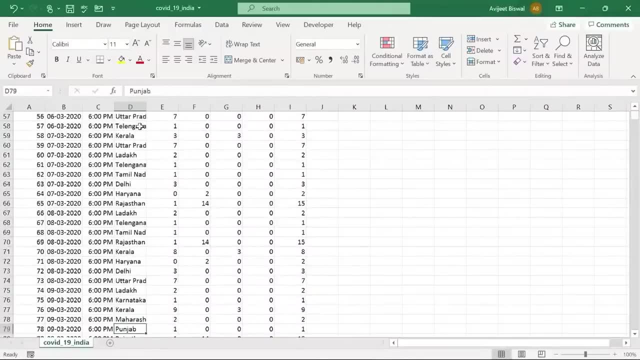 We have the date, We have the time. Then we have the different state names. Let's scroll down. You can see. we have Kerala, Tamil Nadu, Delhi, Haryana, Rajasthan, Ladakh, Punjab, Telangana and other states. 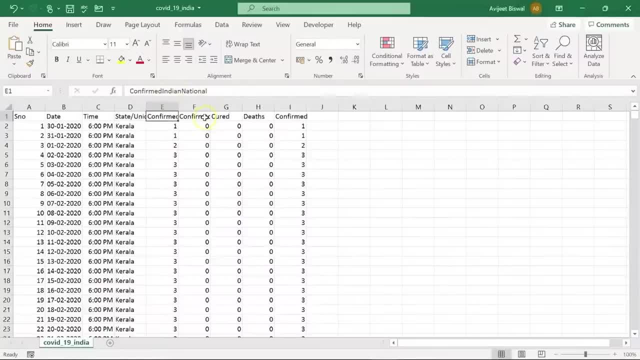 Then we have something called as confirmed Indian national. So actually these two datasets- confirmed Indian national and confirmed foreign national- we won't be using, So in the demo itself will be dropping these two columns. what we are concerned about are the last three columns, the cured cases. 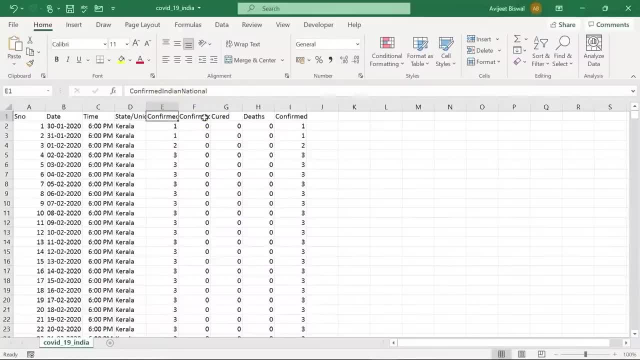 have something called as confirmed Indian national. so actually this two data sets- confirmed Indian national and confirmed foreign national- we won't be using, so in the demo itself. we will be dropping these two columns. what we are concerned about are the last three columns, the cured cases or the 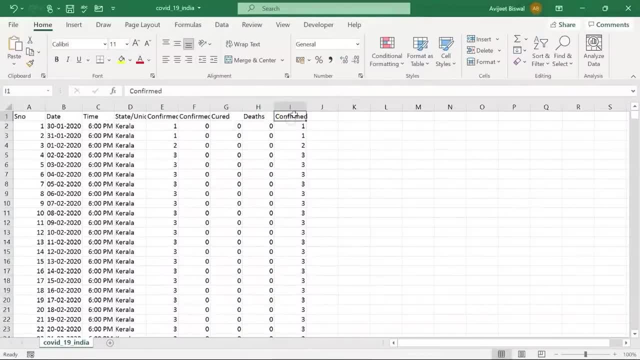 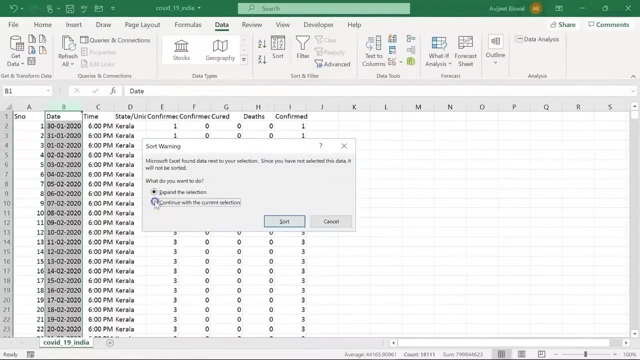 recoveries, the number of deaths reported and then we have the total number of confirmed cases. let me just sort the B column, that is, the date column, so that you have an idea about the recent data we have. I will continue with the current selection and sort it. you can see here. 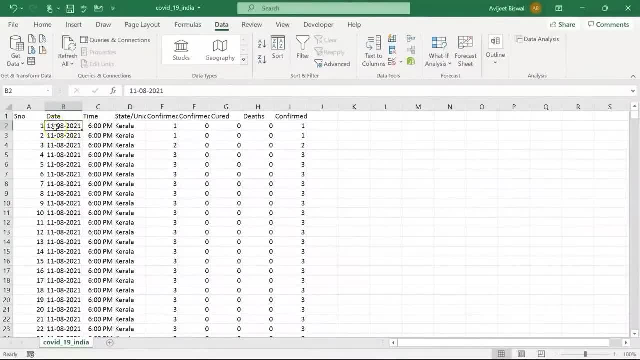 this is till 11th of august 2021, so this data was collected from kegel. it has some discrepancies that we will see in the demo. the data is available for free. we will provide the link to the data sets in the description of the video. 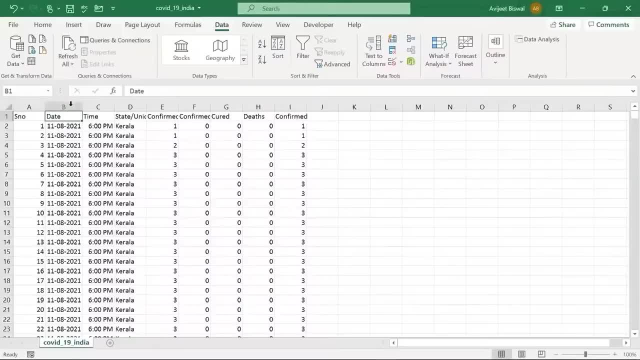 so please go ahead and download them. the visualizations and results that you will see in the demo are based on the data sets that we will be using. we haven't pre-processed the data to remove outliers or any missing values. now, before I jump into the demo, let me show you the 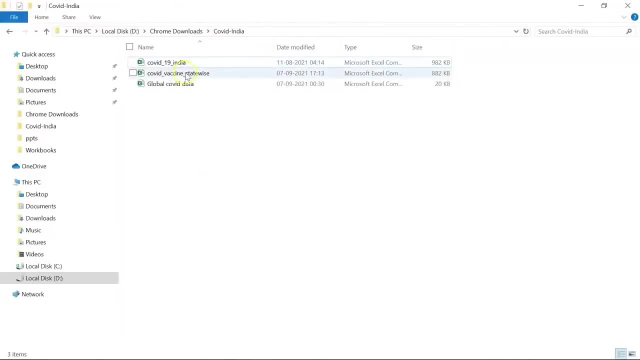 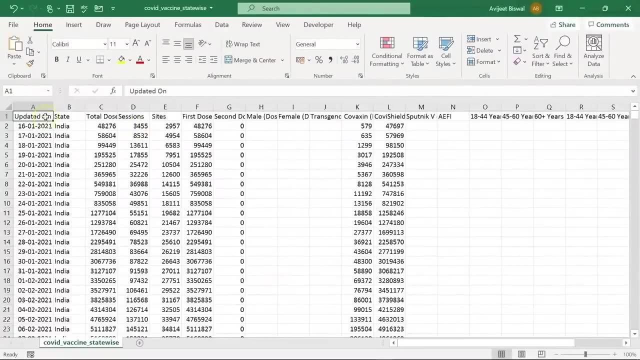 second data set that we are going to use. ok, so covid vaccine state wise is my second data set. let me open it. there you go. so this is the second data set that we will be using in the python project. you can see, we have a column called updated. 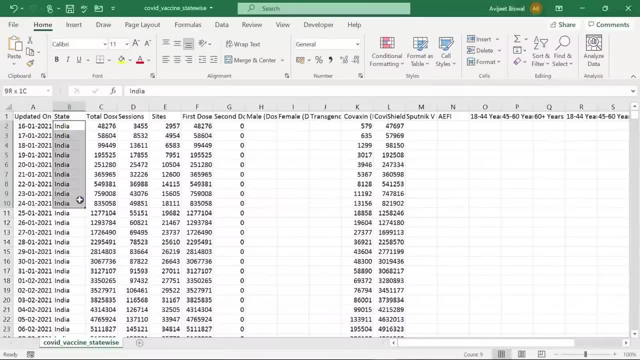 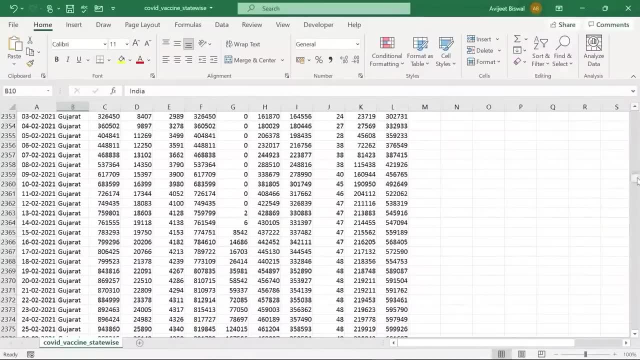 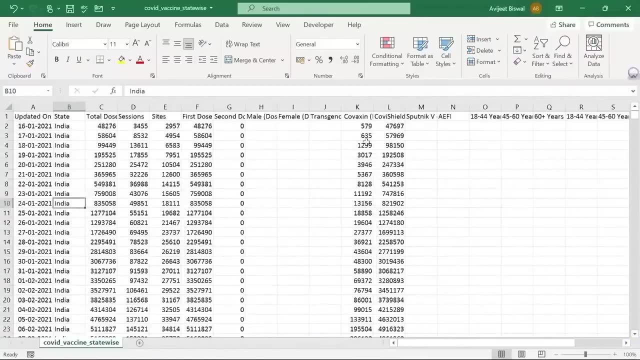 on. then we have the state again. you can see here there are a few discrepancies. here it has taken the country name and not the state name. below you can see there are the different state names and you can also see we have information about the total doses administered we have. 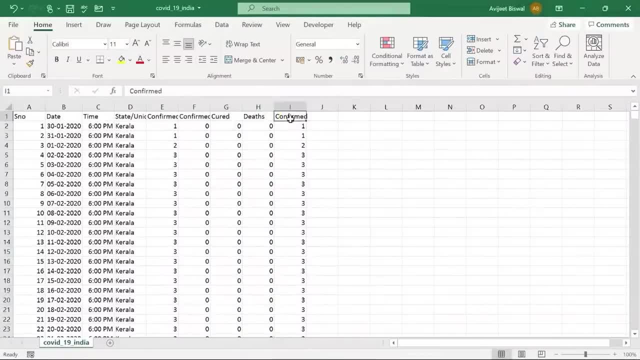 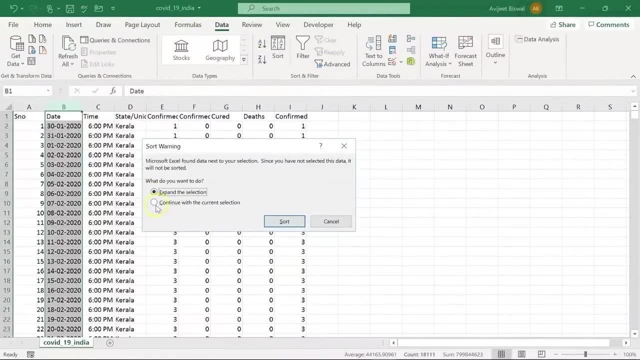 or the recoveries, the number of deaths reported and then we have the total number of confirmed cases. let me just sort the b column, that is, the date column, so that you have an idea about the recent data we have. i'll continue with the current selection and sort it. you can see here. 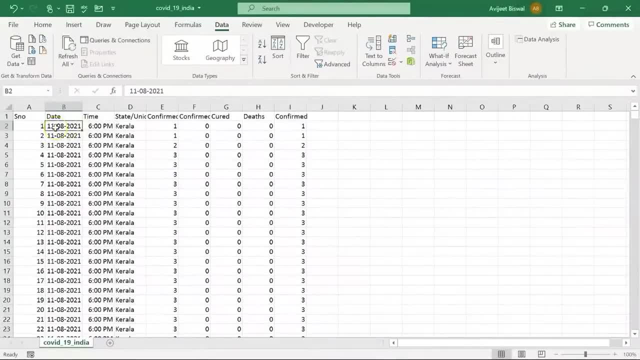 this is till 11th of august 2021, so this data was collected from kegel. it has some discrepancies that we will see in the demo. the data is available for free. we will provide the link to the data sets in the description of the video, so please go ahead and download them. the visualizations and 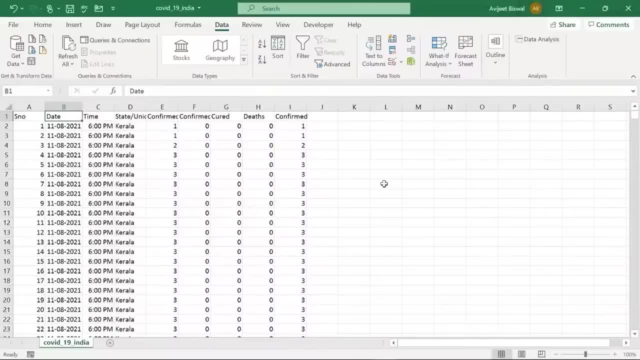 results that you will see in the demo are based on the data sets that we will be using. we haven't pre-processed the data to remove outliers or any missing values. now, before i jump into the demo, let me show you the second data set that we are going to use. 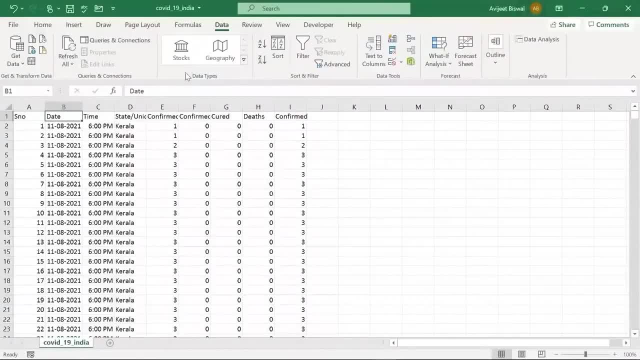 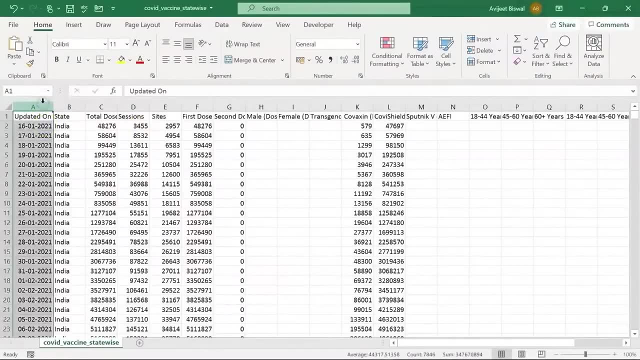 okay, so covet vaccine, state wise, is my second data set. let me open it. there you go. so this is the second data set that we'll be using in the python project. you can see we have a column called updated on. then we have the state again you. 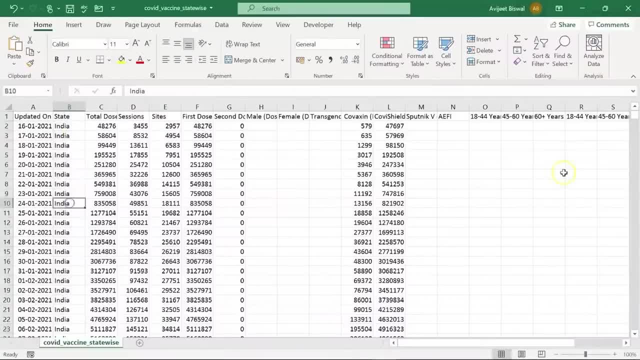 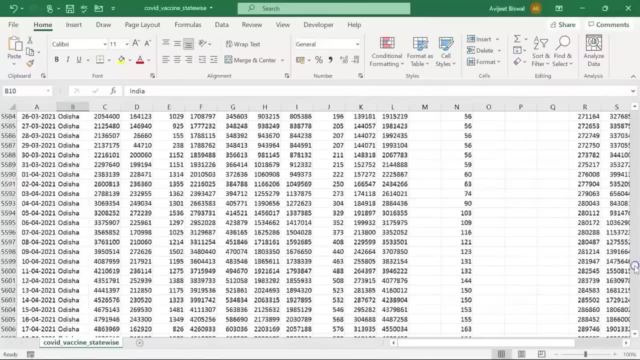 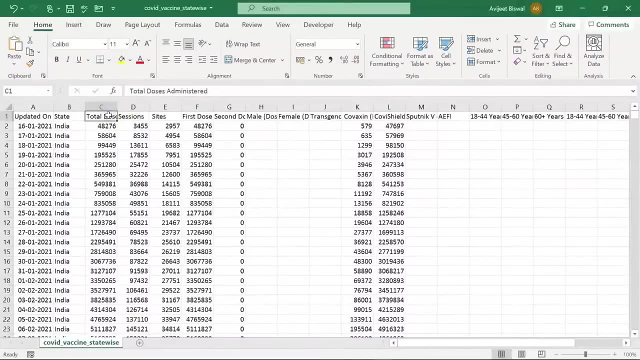 can see here. there are a few discrepancies here. uh, it has taken the country name and not the state. below you can see there are the different state names and you can also see we have information about the total doses administered. we have the sessions sites: first dose administered: 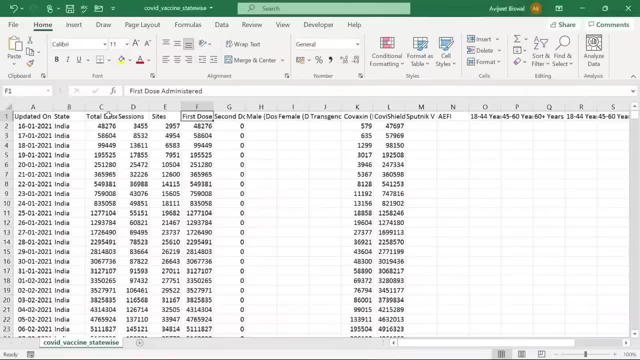 the sessions sites: first dose administered, then we have the second dose, then we have information about male and female doses. you can see here the different vaccines administered: covaxin and covishield. you have sputnik v and here are the different age groups as well. 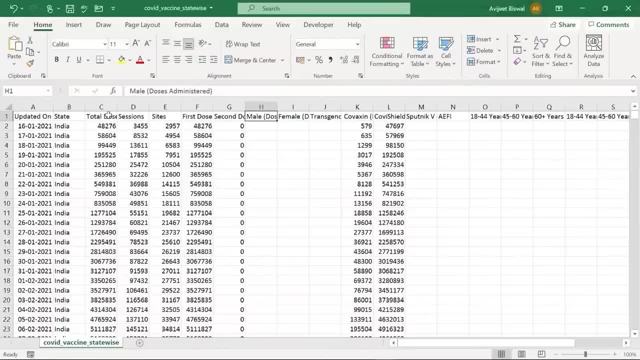 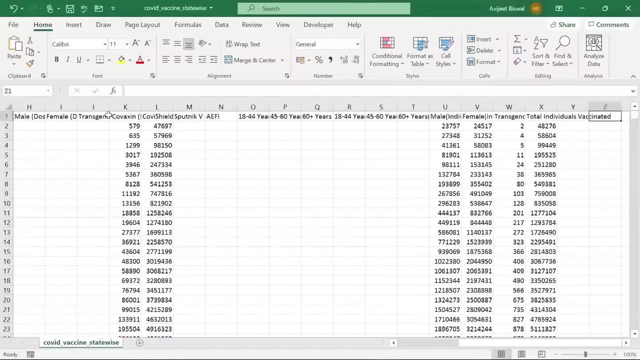 then we have the second dose, then we have information about male and female doses. you can see here the different vaccines administered: covaxin and covishield. you have sputnik v, and here are the different age groups as well. and finally, if you see, we have male individuals. 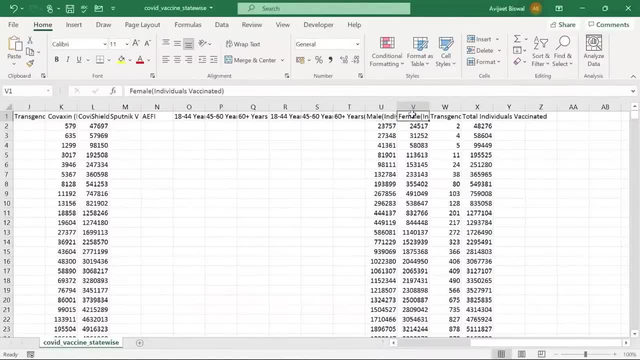 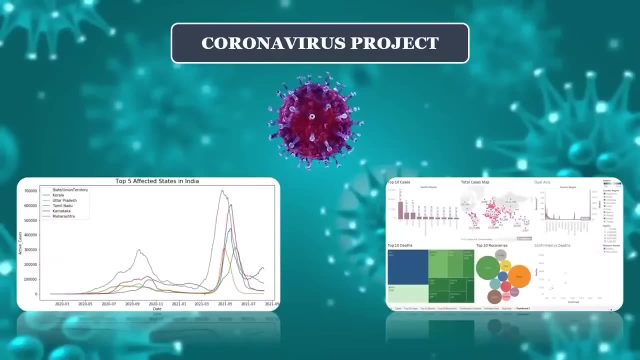 vaccinated, the total number of female individuals vaccinated for a particular day. we have information about transgender individuals vaccinated and, finally, we have the total individuals vaccinated each day. all right, before we jump into the hands-on part, let's have a look at the second quiz in this project. 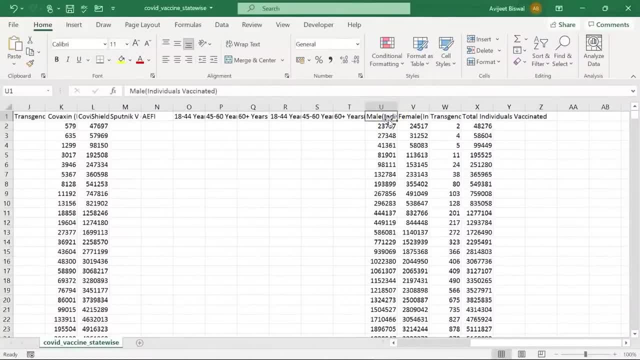 and finally, if you see, we have male individuals vaccinated, the total number of female individuals vaccinated for a particular day, we have information about transgender individuals vaccinated and, finally, we have the total individuals vaccinated each day. alright, before we jump into the hands on part, let's have a look at the second. 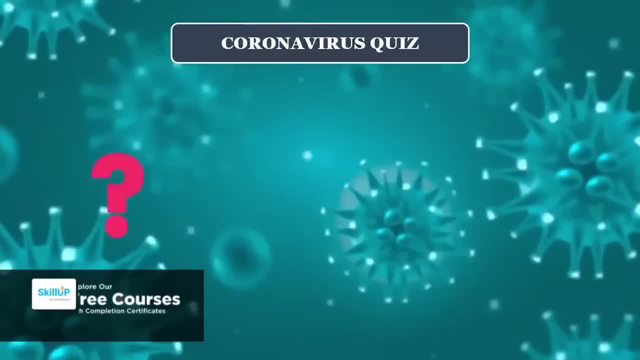 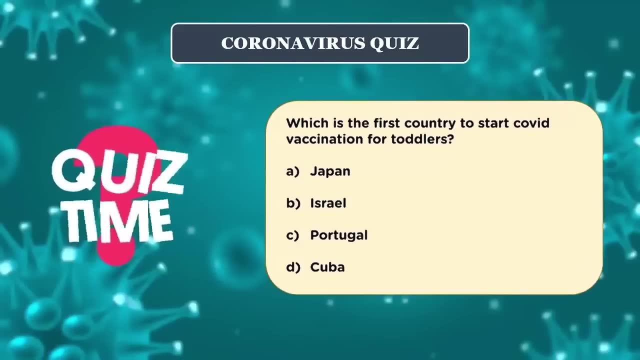 quiz in this project. so here is the second quiz question: which is the first country to start covid vaccination for toddlers? is it a- japan, b- israel, c- portugal or is it d- cuba? this is a very recent development that took place if you watch daily news updates. 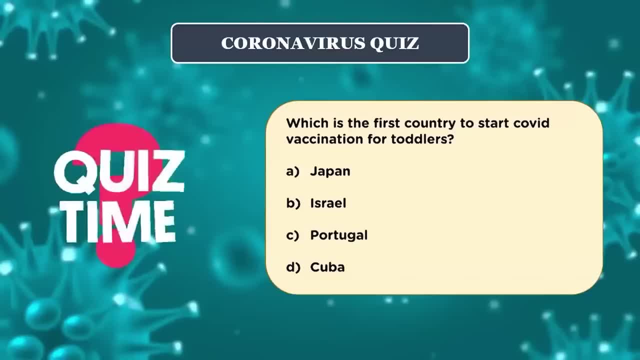 on coronavirus. you will be definitely able to answer the question. please give it a try and put your answers in the comment section of the video. it is really important for our viewers to know the right answer. alright, so now let's begin with our demo. so i am on my. 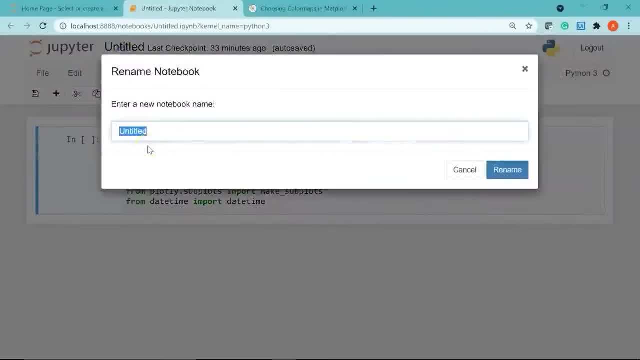 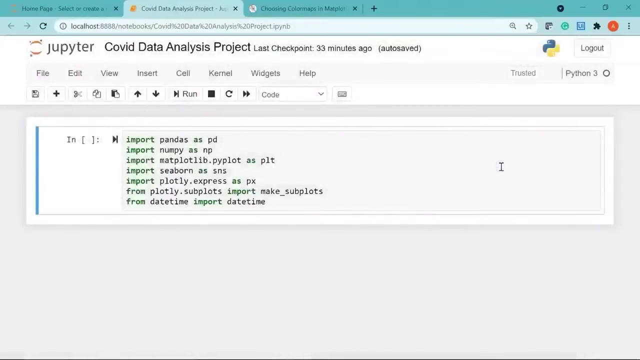 jupyter notebook. so the first project we are going to use, python jupyter notebook. i will just rename this notebook as covid data analysis project. i will click on rename alright. so first and foremost, we need to import all the necessary libraries that we are going to use. so first i am importing pandas. 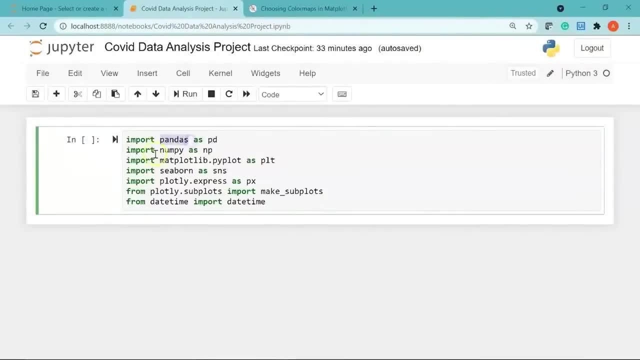 as pd. this is for data manipulation. then we have numpy, as np. numpy is used for numerical computation. then we are importing matplotlib, seaborn and plotly. these three libraries will be used for plotting our data and creating interesting visualizations. finally, i am also importing my datetime function. 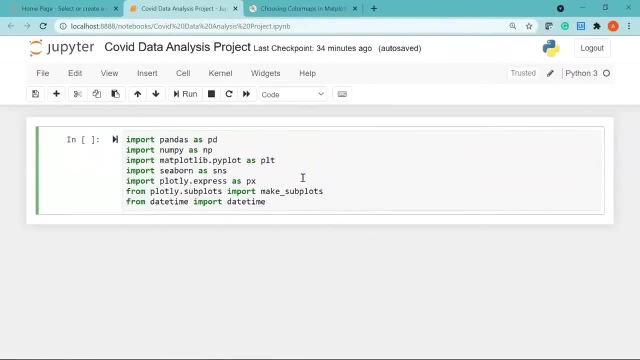 alright, so i will hit shift enter to run the first cell. now it's time to load our first dataset, which is related to the covid 19 cases in india for the different states and union territories. so i will create a variable called covid, underscore df- df is for data frame. 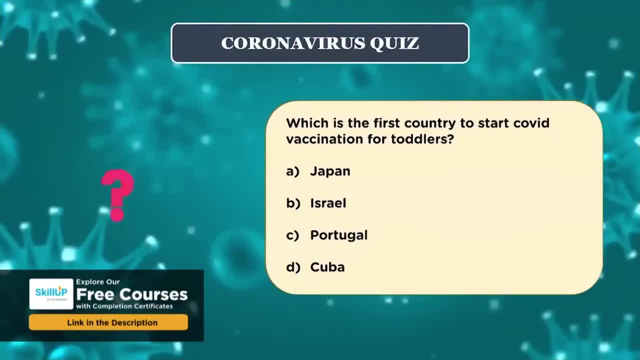 so here is the second quiz question: which is the first country to start covid vaccination for toddlers? is it a- japan, b- israel, c- portugal or is it d- cuba? this is a very recent development that took place. if you watch daily news updates on coronavirus, you will be definitely able to answer. 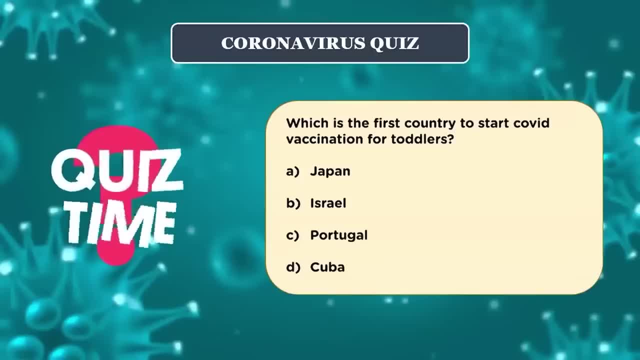 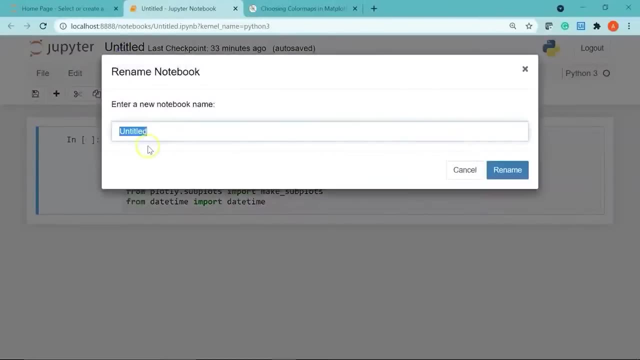 the question. please give it a try and put your answers in the comment section of the video. it is really important for our viewers to know the right answer. all right, so now let's begin with our demo. so i am on my jupyter notebook, so the first project we 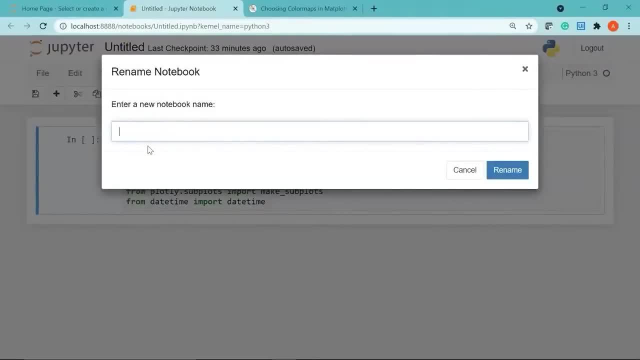 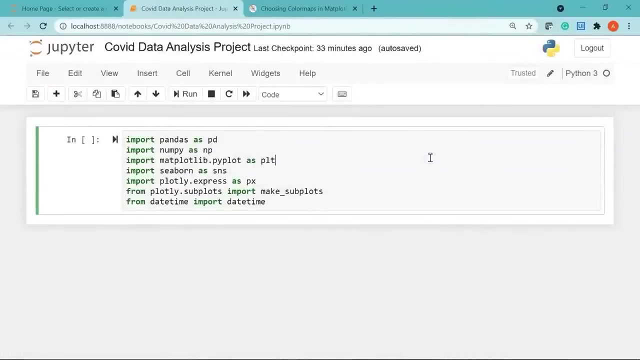 are going to use python jupyter notebook. i'll just rename this notebook as covid data analysis project. i click on rename, all right. so first and foremost we need to import all the necessary libraries that we are going to use. so first i'm importing pandas spd- this is for data manipulation- then we 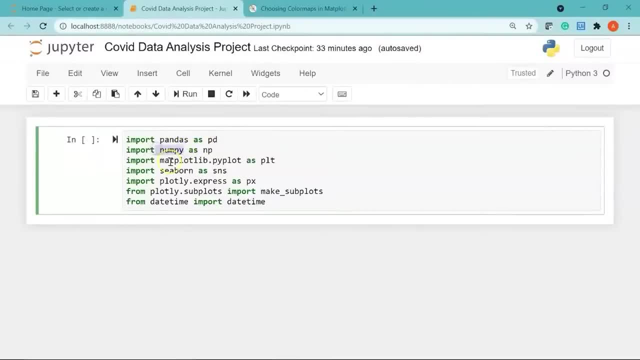 have numpy, as np numpy is used for numerical computation. then we are importing matplotlib, seaborn and plotly. these three libraries will be used for plotting our data and creating interesting visualizations. finally, i'm also importing my date time function. all right, so i'll hit shift enter. 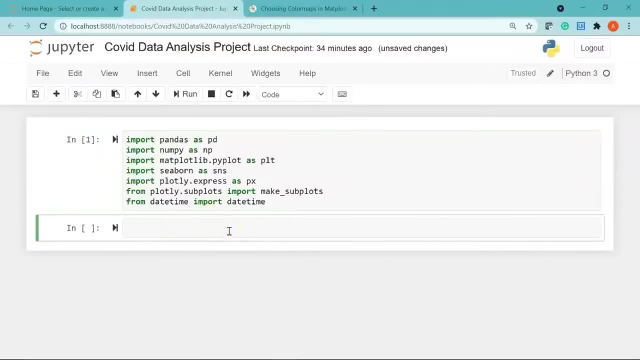 then i'll hit call to run the first cell. now it's time to load our first data set, which is related to the covid-19 cases in india for the different states and union territories. so i'll create a variable called covid, underscore df- df is for data frame. 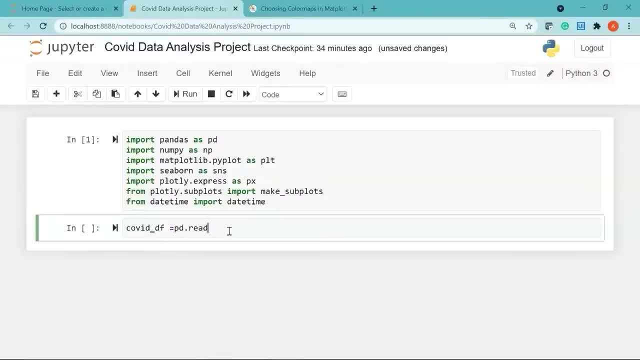 i'll use my pandas library and then give the read underscore csv function. since sets are CSV files and inside double quotes, I will pass in the location where my data sets are present. so I just copy this location, I'll paste it here, will change the backslash to forward slash and after that I am going to give my 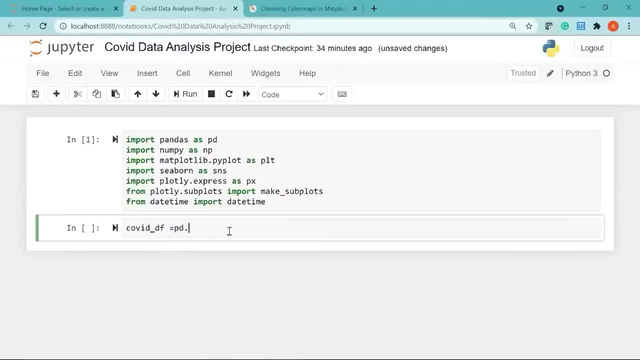 i will use my pandas library and then give the read underscore csv function. since our datasets are csv files and inside double quotes, i will pass in the location where my datasets are present. so i will just copy this location. i will paste it here. we will change the back. 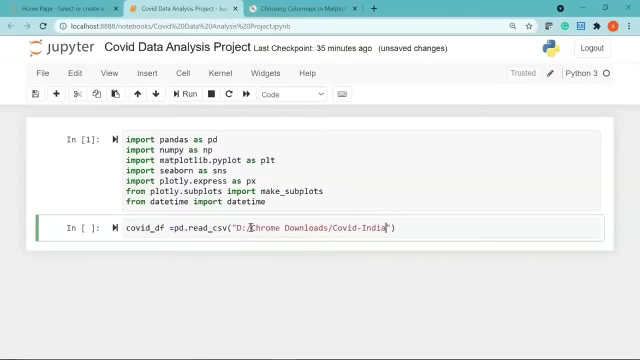 slash to forward slash and after that i am going to give my file name, followed by the extension of the file. i will say covid 19, india dot csv. let's go ahead and run it. alright, now to see the first few rows of the data frame, i am going to use the head. 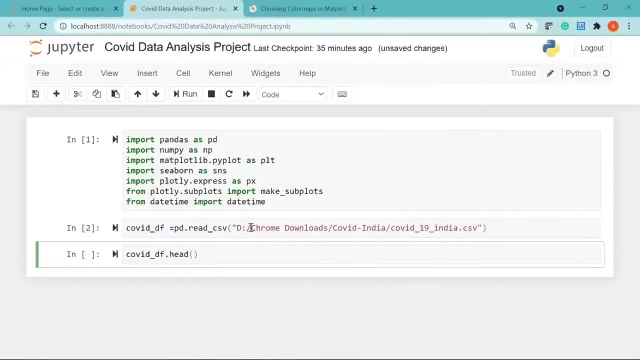 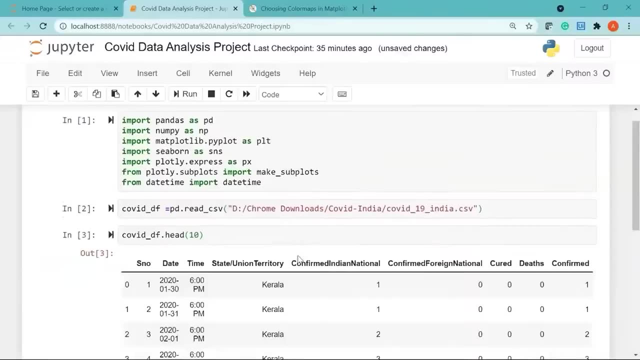 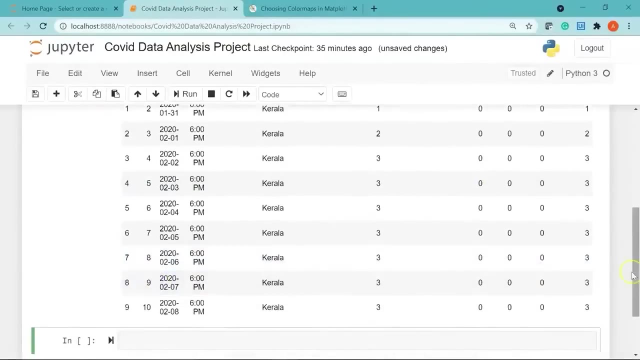 function. i will say head and within brackets, let's say i will pass in 10, which means i want to see the first 10 rows of data. if i run it there, you go here. you can see from 0 till 9. so we have 10. 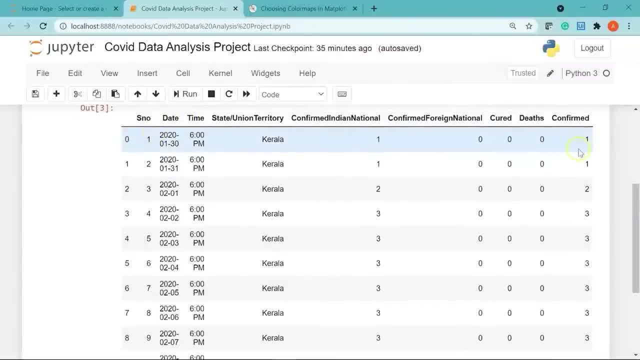 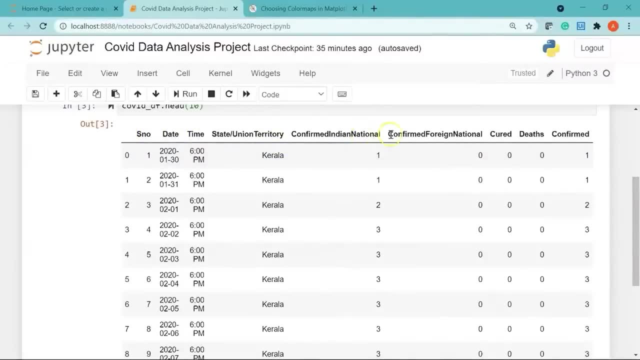 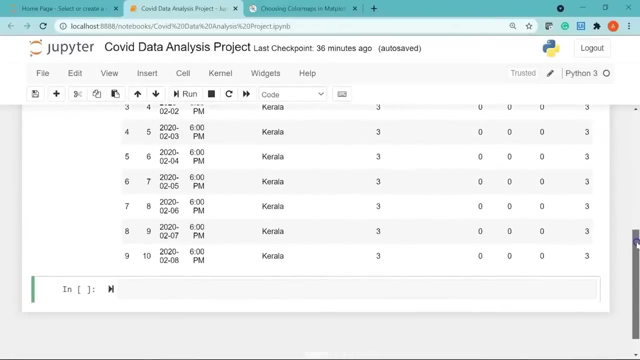 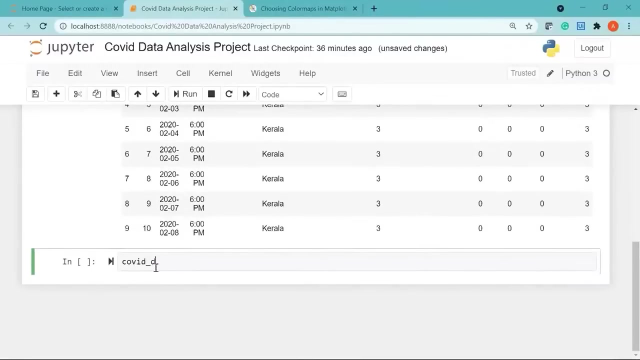 rows of information and these are the different column names. you have s number, date, time, state or union territory. then you have confirmed indian national, confirmed foreign national, cured cases, deaths reported and the confirmed cases. alright. now moving ahead, let's use the info function to get some idea about. 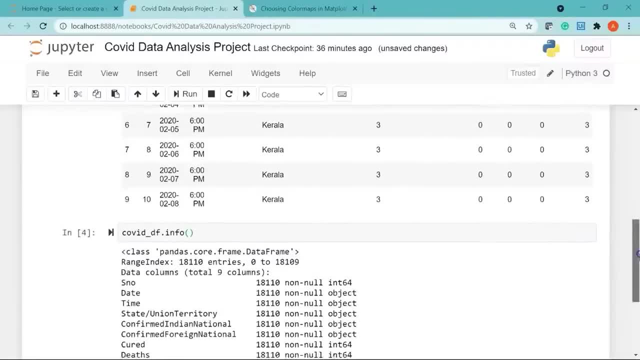 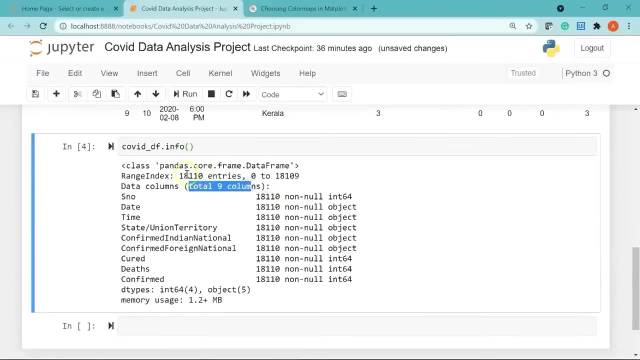 a data set. if i run it, you can see here. it gives us the total number of columns- we have 9 columns- the total number of entries or the rows. we have 18110 rows of information, starting from 0 till 18109. you see here the different types of 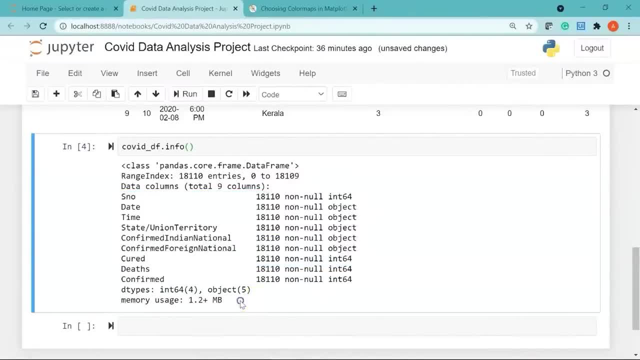 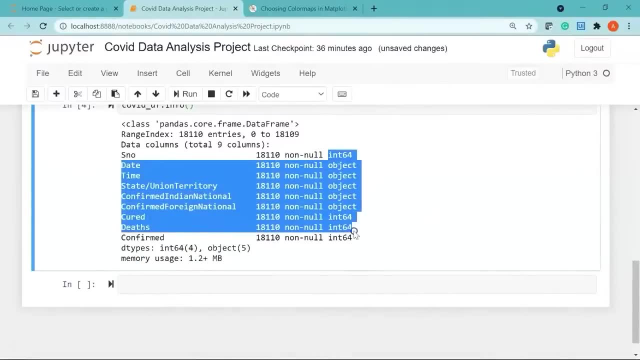 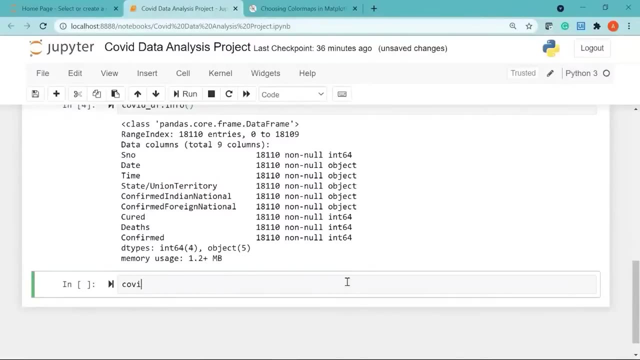 variables or column names that we have. then it has information about the memory usage as well and this side, you can see the data types. cool. now we will use another very important function, which is to get some idea about statistical analysis, the basic statistics about your data set for. 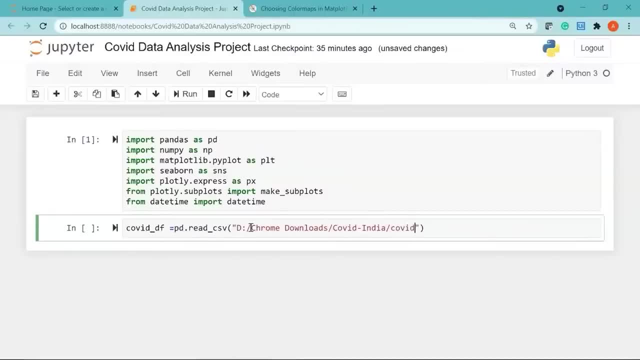 file name, followed by the extension of the file as a COVID-19 India dot CSV. let's go ahead and run it all right now. to see the first few rows of the data frame, I am going to use the head function. I'll say head and within. 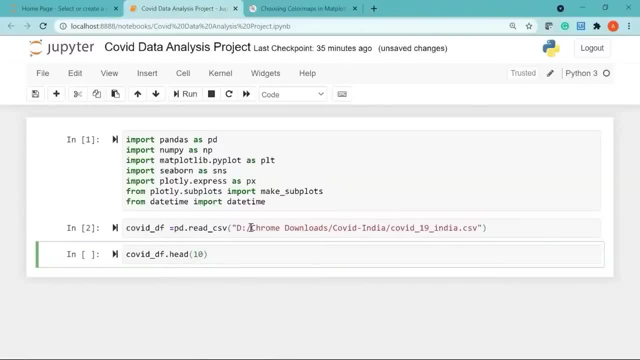 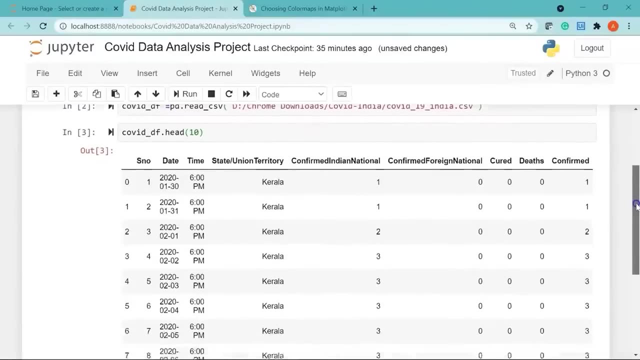 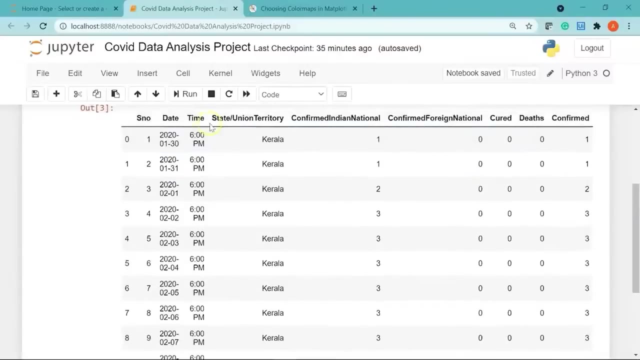 brackets. let's say I'll pass in 10, which means I want to see the first 10 rows of data. if I run it there, you go here. you can see from 0 till 9. so we have 10 rows of information and these are the different. 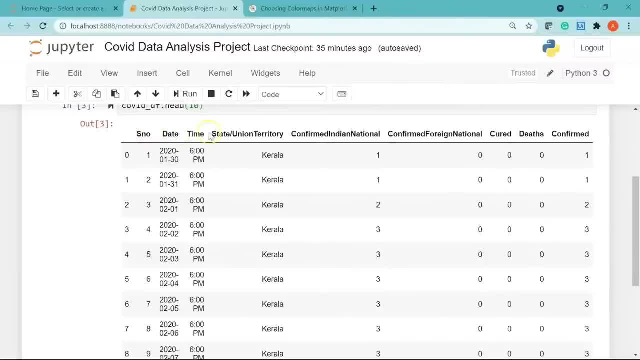 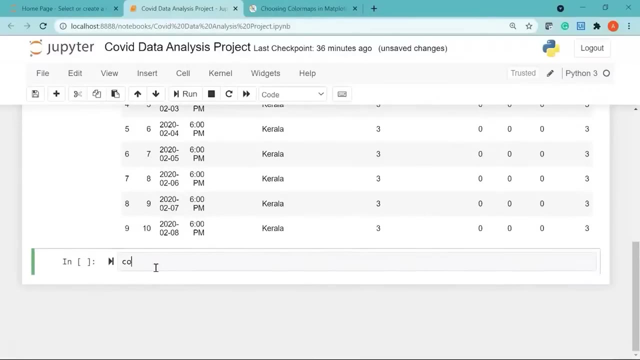 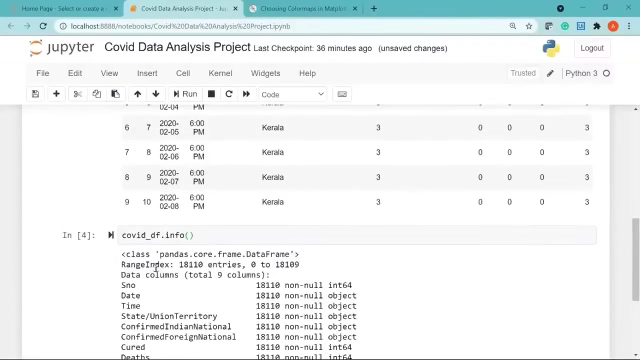 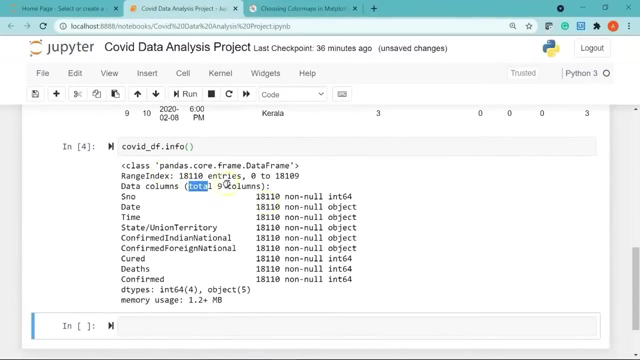 column names. you have s number, date time, state or union territory. then you have confirmed Indian national, confirmed foreign national, cured cases, deaths reported and the confirmed cases. all right, moving ahead, let's use the info function to get some idea about a data set. if I run it, you can see here. it gives us the total number of columns we 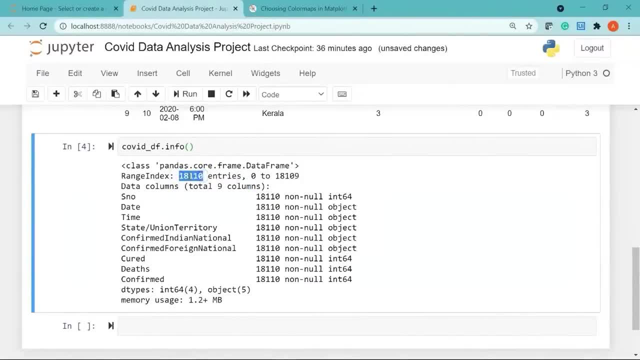 have 9 columns. the total number of entries for the rows. we have eighteen thousand hundred and ten rows of information, starting from zero till eighteen thousand one hundred and nine. you see here the different types of prayer names that we have. then it has information about the memory usage as 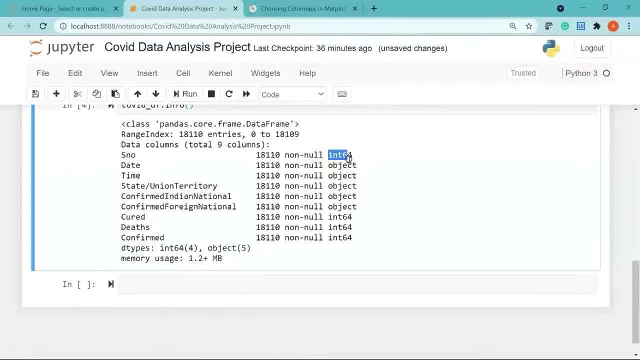 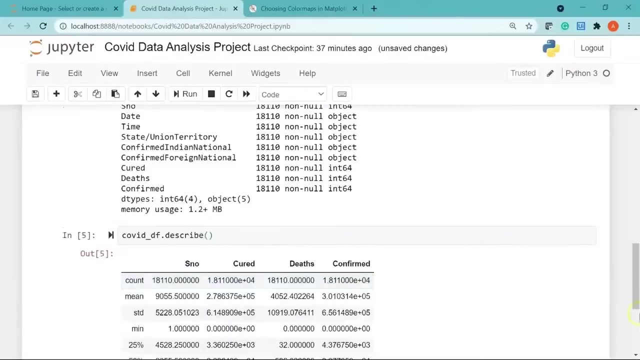 well, and this side, you can see the data types. cool, now we'll use another very important function, which is to get some idea about statistical analysis, the basic statistics about your data set. for that I will be using the describe function. okay, so if you can see, here the describe function is for numerical. 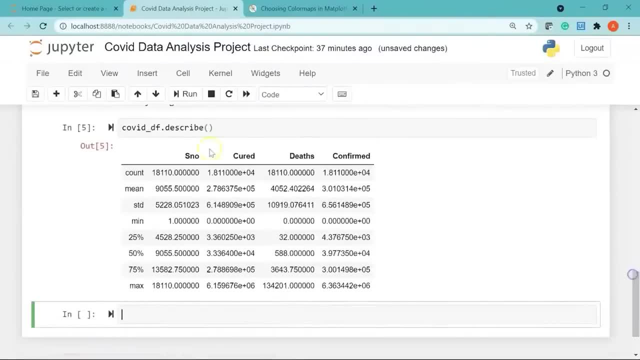 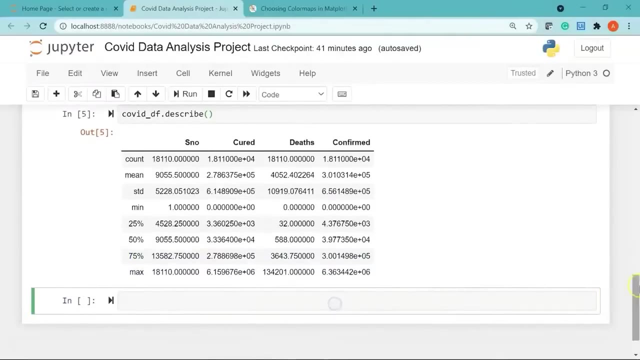 columns only and you have the measures, such as count, the mean standard deviation, maximum, minimum, the 25th percentile, 50th percentile and the 75th percentile value. okay, now let's move ahead and import the data set for the data set function, and then we will be using the data set function. 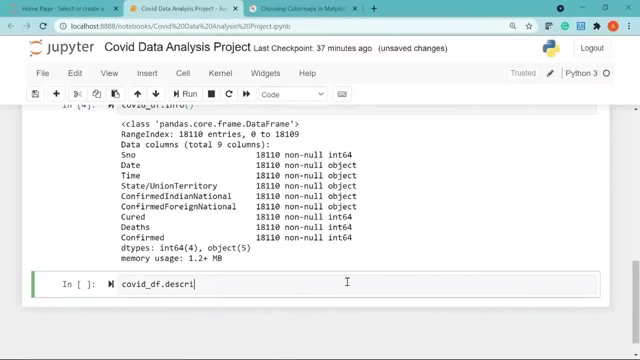 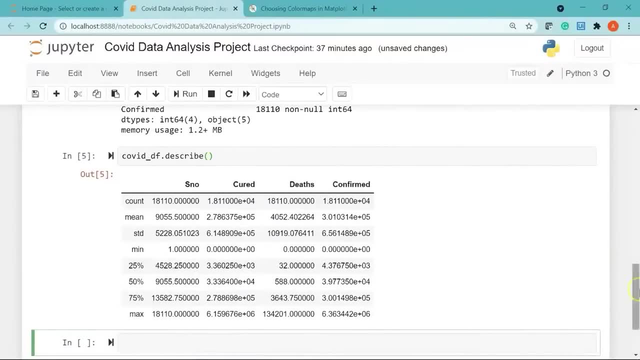 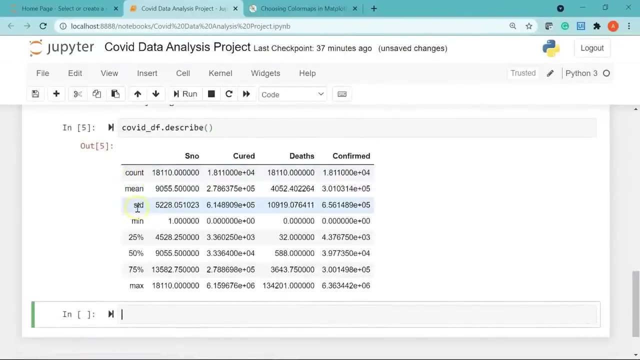 that i will be using the describe function. ok, so, if you can see, here the describe function is for numerical columns only and you have the measures such as count, the mean, standard deviation, maximum minimum, the 25th percentile, 50th percentile and the 75th percentile value. 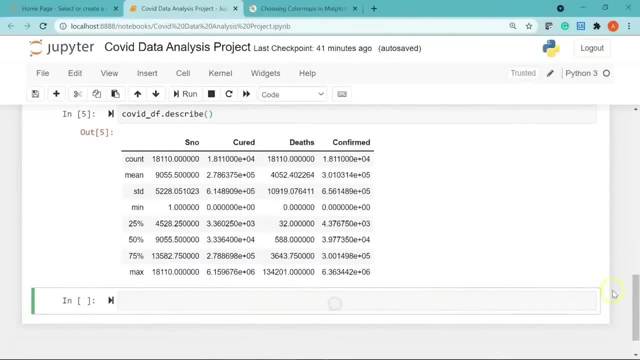 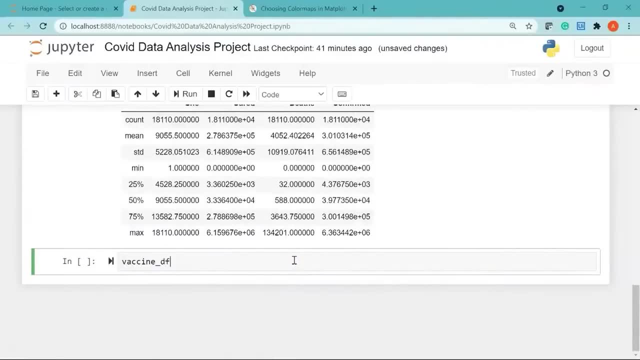 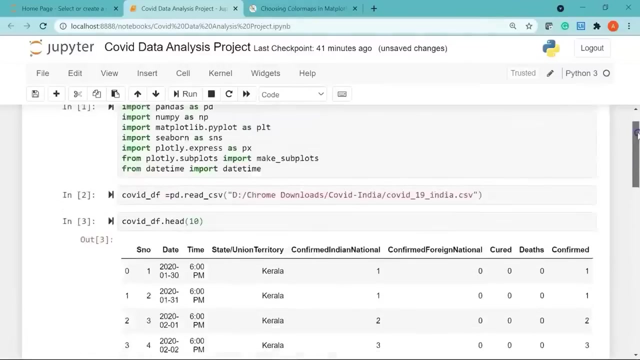 ok, now let's move ahead and import the second data set, which is related to vaccination. so i will create a variable called vaccine underscore df. i will write pd dot read underscore csv function which is present in pandas library. i will move to the top and i will copy the 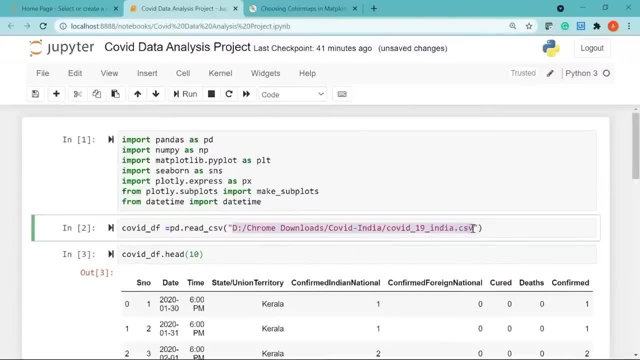 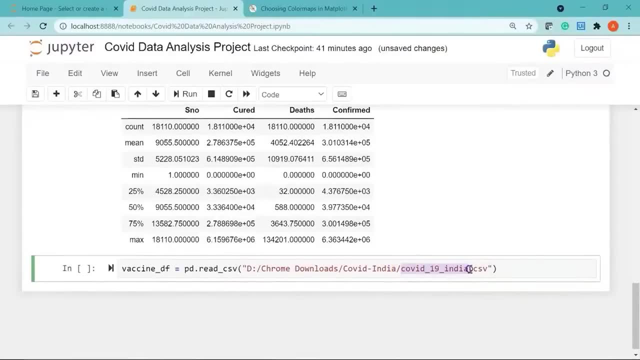 file location and we will change the name of the file. copy this and let me paste it here: and instead of covid underscore 19 underscore india, i am going to say covid underscore- vaccine- underscore state- wise. ok, so this is the data set that we saw: covid underscore- vaccine underscore state. 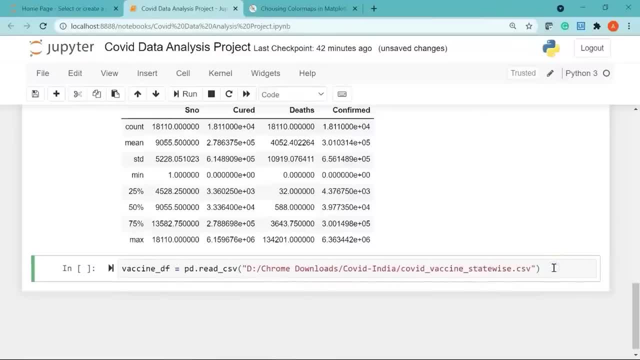 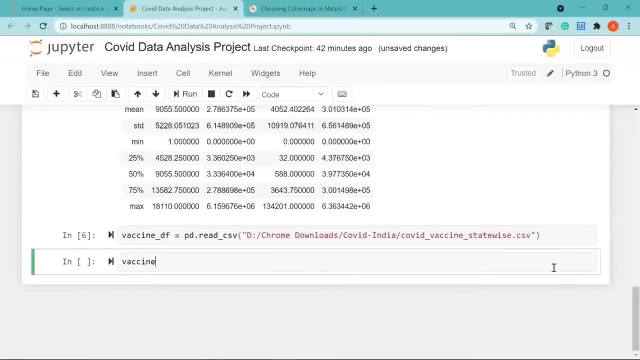 wise. alright, let me run it cool and let's display the first 7 rows of information from this data frame. i will be using the head function and inside the function i will pass in 7. there you go. so here you can see we have from 0. 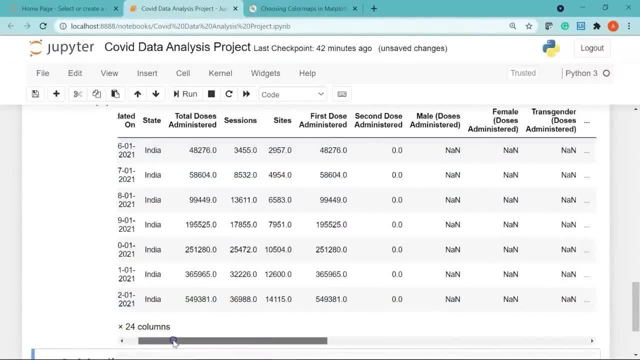 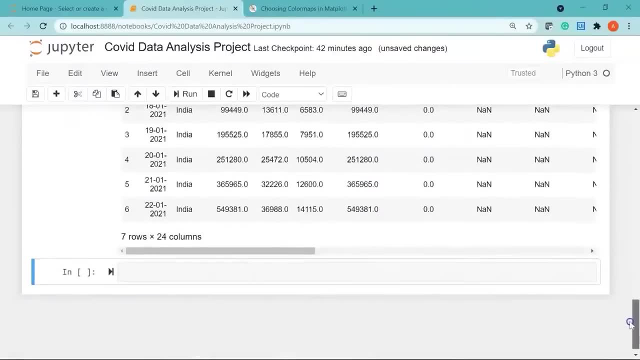 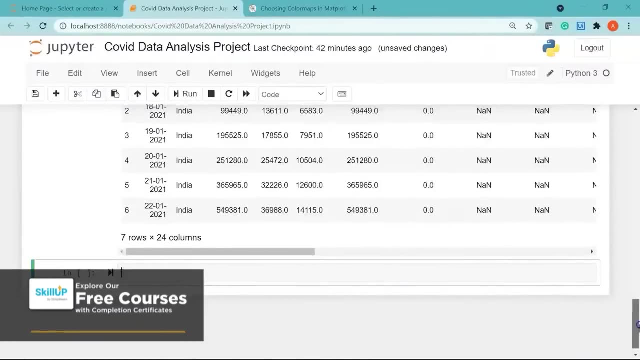 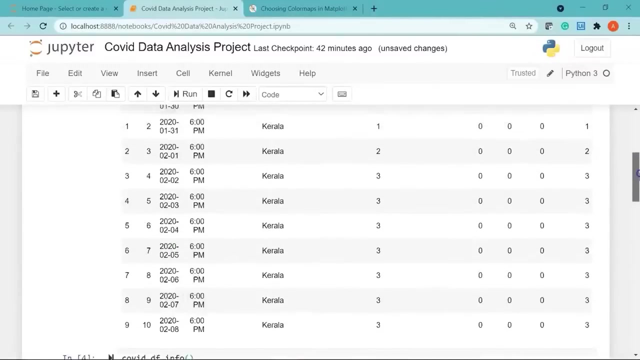 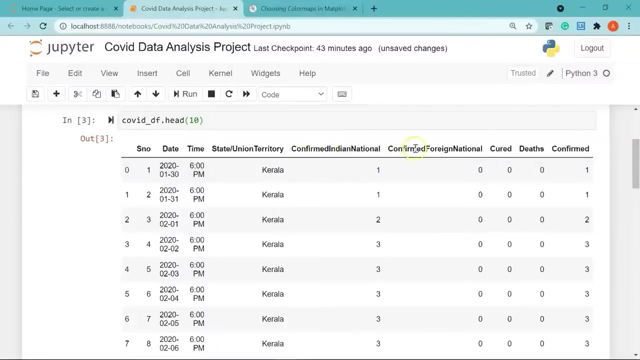 till 6, there are total 24 columns. a lot of them have null values. you can see here: alright, now, from the first data set, which is the covid underscore df data frame, we will be dropping a few unnecessary columns, such as the time column. confirmed. indian national and confirmed. 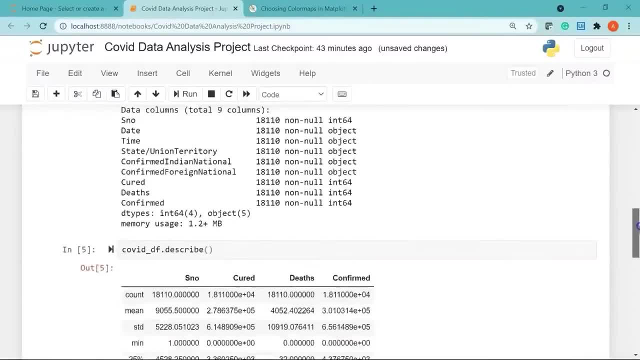 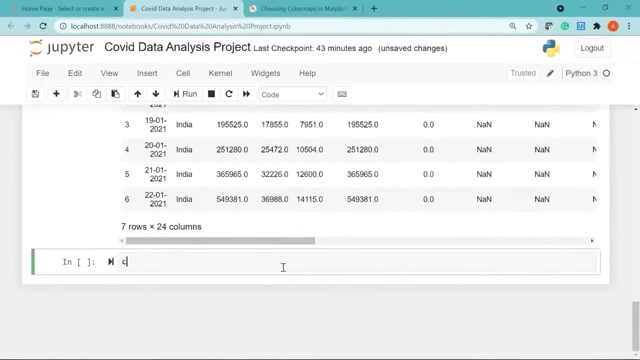 foreign national as well as the s number. we don't need these columns, so it's better to learn how to drop the columns for our analysis. so i will say covid, underscore, df, dot. i will use the drop function and, within square brackets, i will pass in the 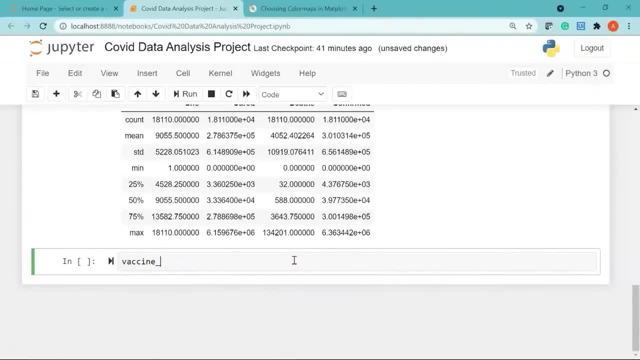 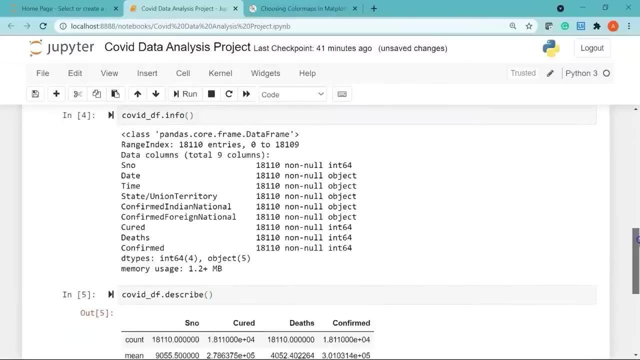 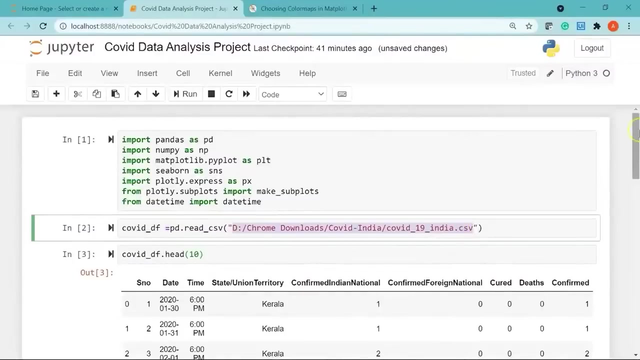 second data set which is related to vaccination. so I'll create a variable called vaccine. underscore DF, I'll write PD dot read. underscore CSV function, which is present in pandas library. I'll move to the top and I'll copy the file location and we'll change the name of the file. copy this and let me paste it. 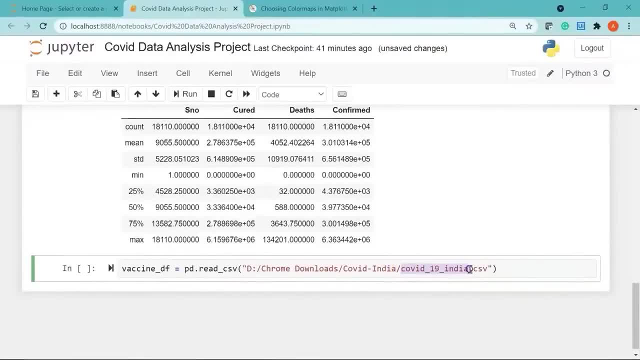 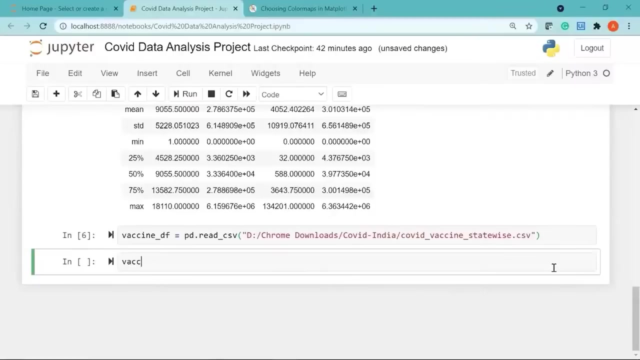 here, and instead of of kovat underscore 19 underscore India, I'm going to say kovat underscore vaccine underscore state wise. okay, so this is the data set that we saw: kovat underscore vaccine, underscore state wise. all right, let me run it cool and let's display the. 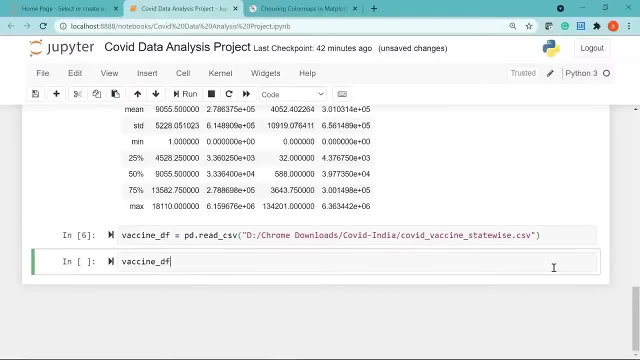 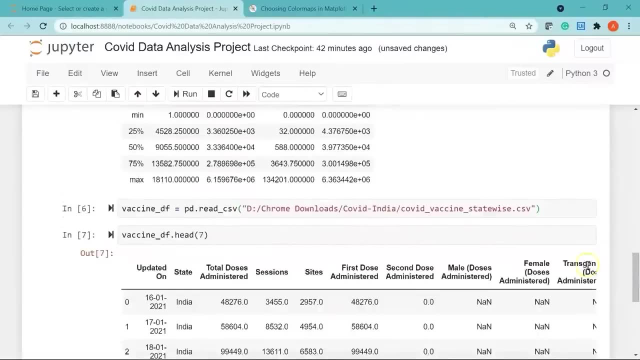 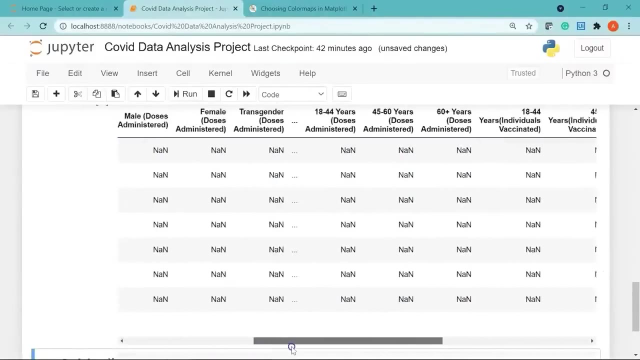 first seven rows of information from this data frame. I'll be using the head function and inside the function I'll pass in seven. there you go. so here you can see we have from 0 till 6. there are total 24 columns. a lot of them have null. 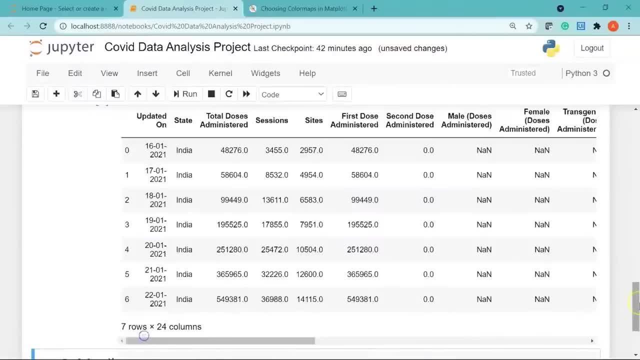 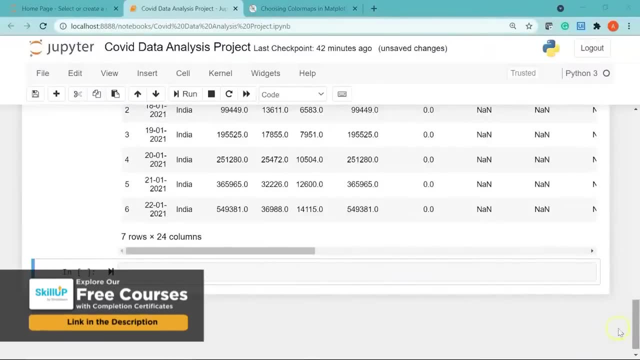 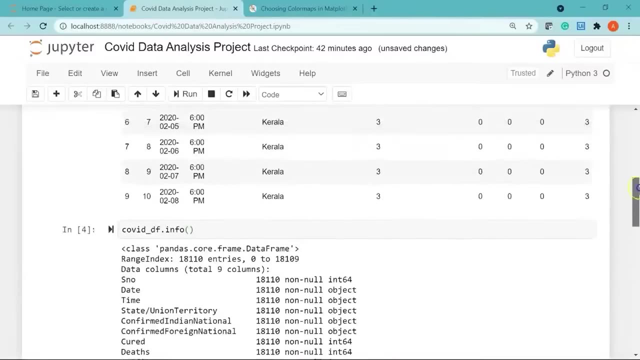 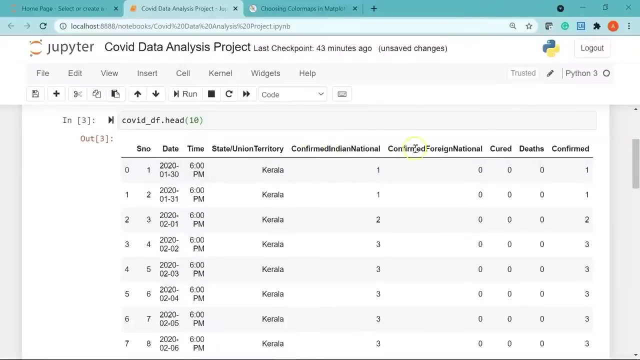 values. you can see here all right now from the first data set, which is the kovat underscore DF data frame, we'll be dropping a few unnecessary columns, such as the time column, confirmed Indian national and confirmed foreign national, as well as the s number. we don't need these columns, so it's. 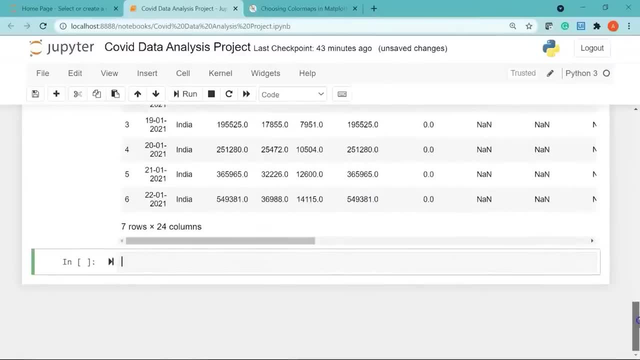 better to learn how to drop the columns for our analysis. so I'll say kovat, underscore, DF, dot. I'll use the drop function and within square brackets I'll pass in the column names. the first is s number. you give a comma within double quotes. I'll 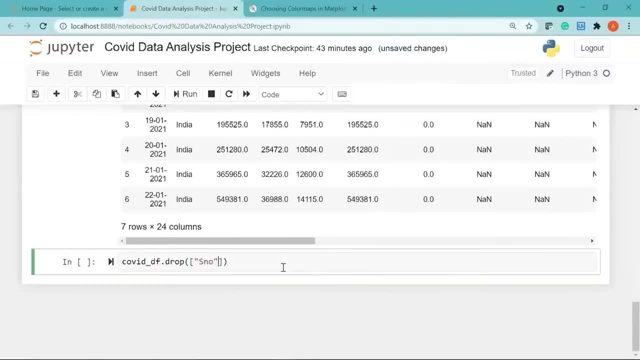 column names. the first is s number. i will give a comma. within double quotes. i will say the next column is time. my third column that i want to drop is confirmed indian national. give another comma within double quotes. i will say confirmed foreign national. outside the brackets, i will give another comma and. 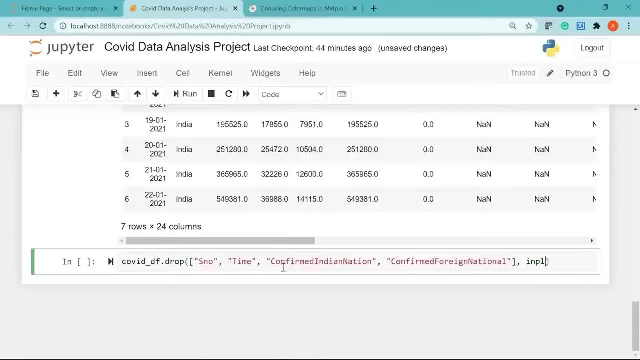 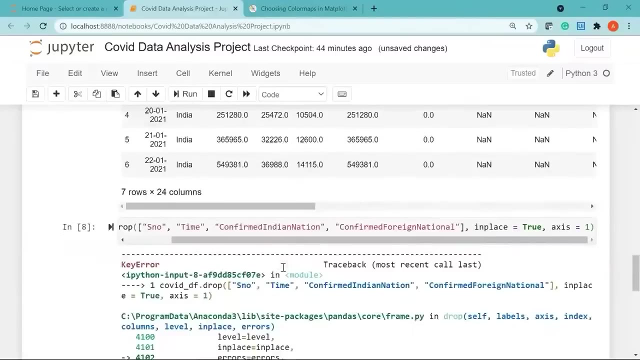 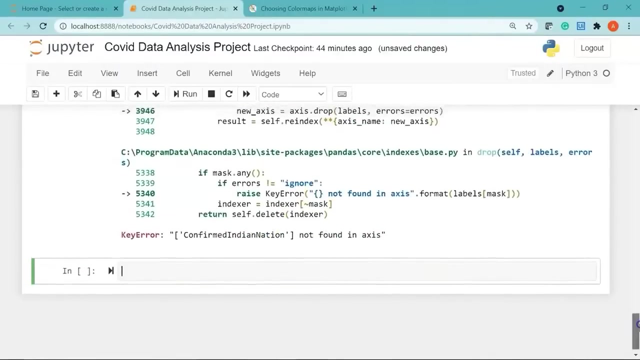 pass in my next argument: that is in place, equal to, i will say true. i will give another comma and say axis equal to one. let's run it. ok, it has thrown an error. let's debug. the error says confirmed indian. ok, it should be indian national and not indian nation. 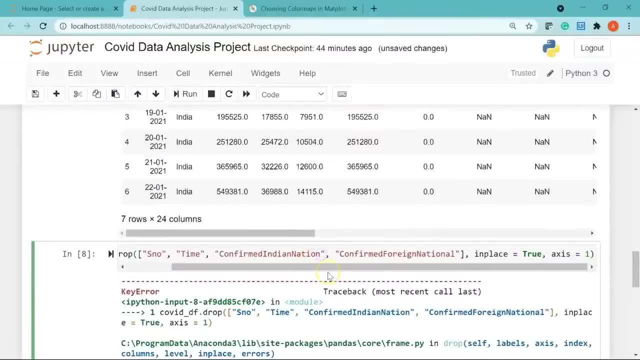 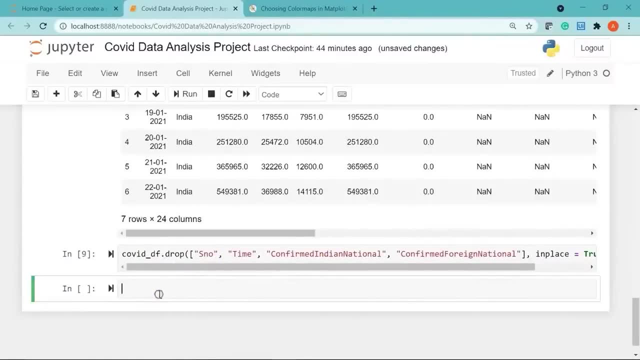 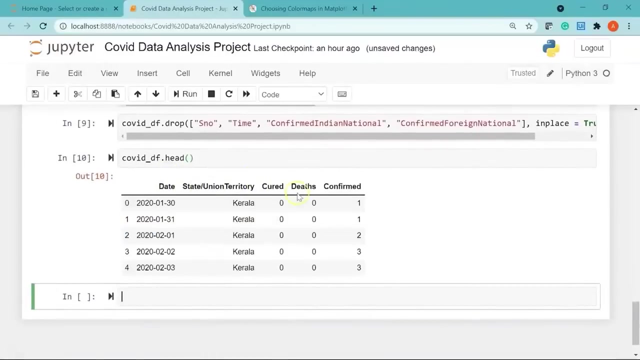 i will just mention it as national. we will run it again. ok, now we have removed these four columns, let me show you the data set now. there you go. so we have only the date, column, state or union territory, cured deaths and confirmed. now let's see how you can. 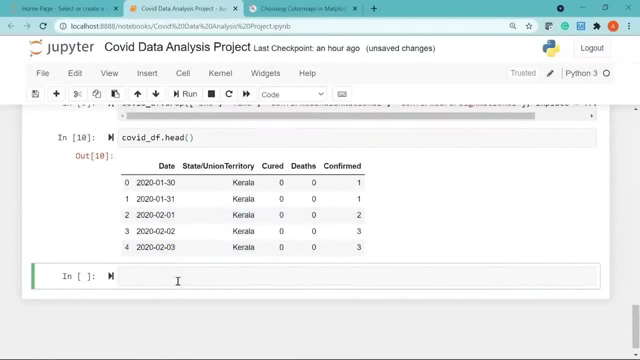 change the format of the date column. for that you have the function called to date time. i will say covid, underscore df. i will pass in my column name that is date. i will say equal to pd dot. i will use the pandas function, that is to underscore date time. 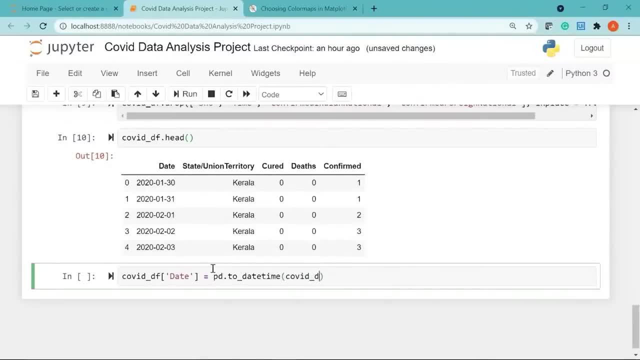 ok, i will say covid, underscore df, which is my data frame name. pass in my variable, which is date, give a comma, and i will use my argument. that is format equal to. i will say percentage y. give a dash. say percentage m. give another dash and say percentage. 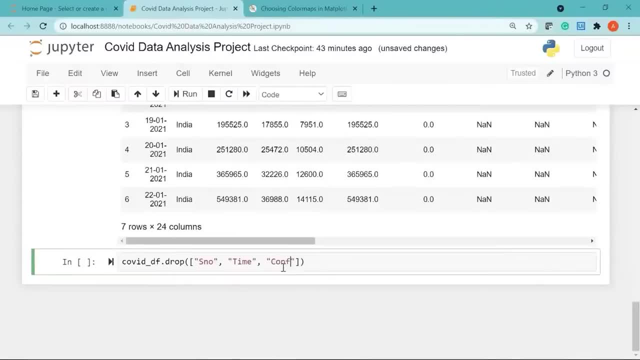 see. the next column is time. my third column that I want to drop is confirmed Indian national. give another comma within double quotes. I'll see confirmed foreign national outside the square brackets. I'll give another comma and pass in my next argument that is in place, equal to. I'll say: true, you give. 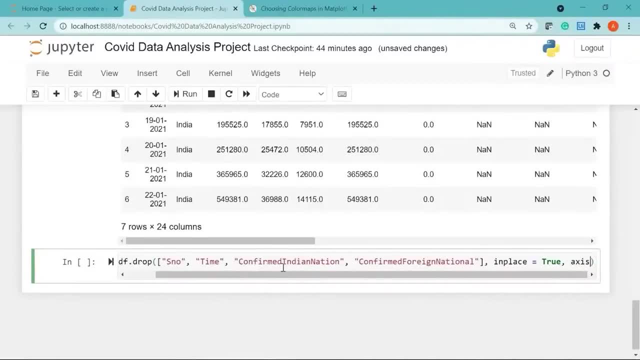 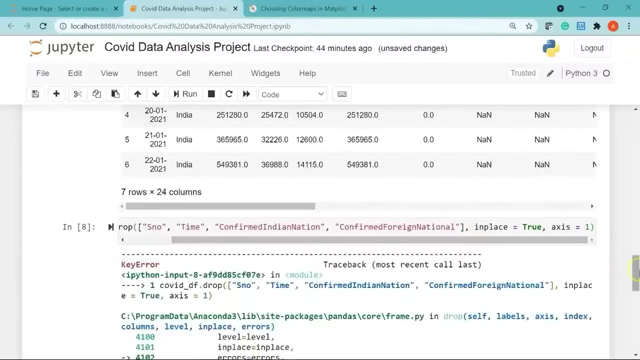 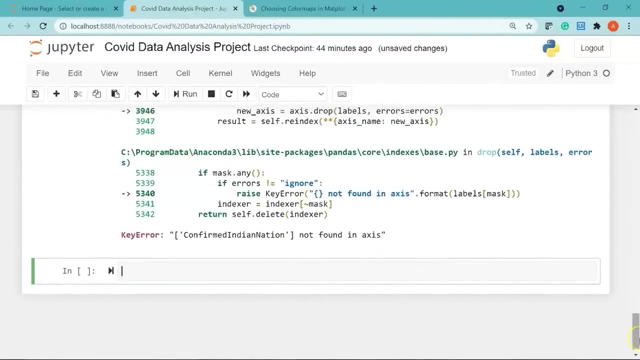 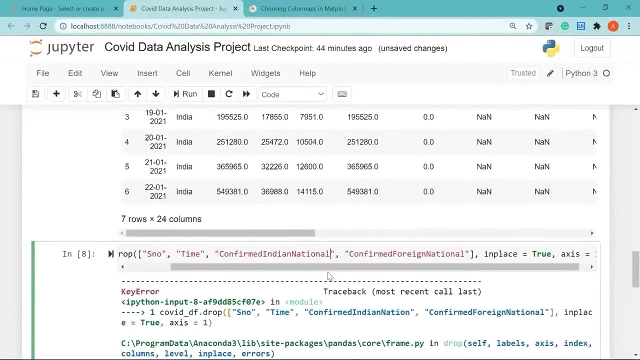 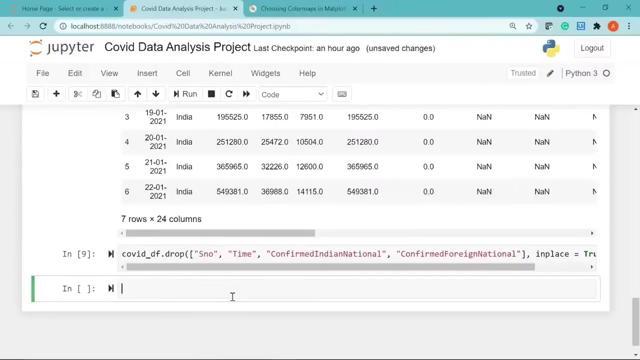 another comma and say: axis equal to 1, let's run it. okay, it has thrown an error. let's debug. the error says: confirmed Indian. okay, it should be Indian national and not Indian nation. I just mention it as national. will run it again. okay, now we have removed these four. 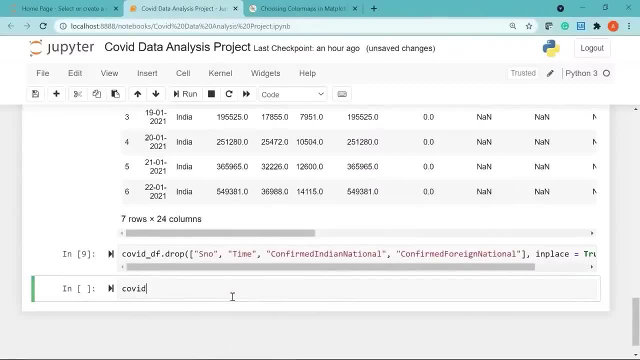 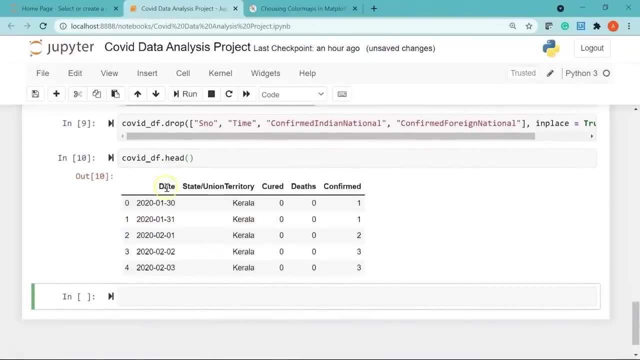 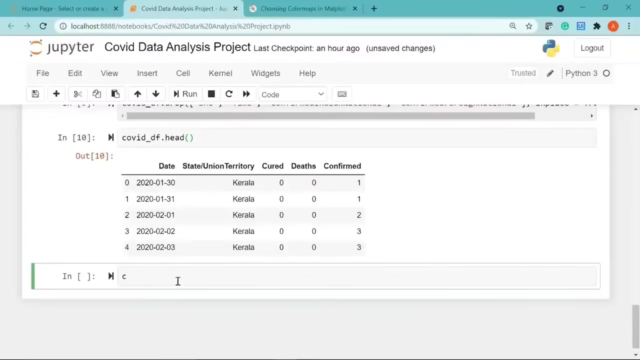 columns. let me show you the data set now. there you go. so we have only the date column: state or union territory, cured deaths and confirmed. now let's see how you can change the format of the date column. for that you have the function called to date time. I'll say kuvet. 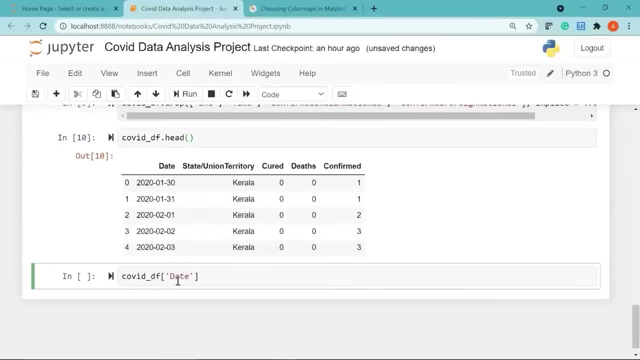 underscore DF, will pass in my column name. that is date. I'll say equal to pd dot. i'll use the pandas function, that is 2 underscore date time. i'll say covid. underscore df, which is my data frame name. pass in my variable, which is date. give a comma and i'll use my argument. that is format. 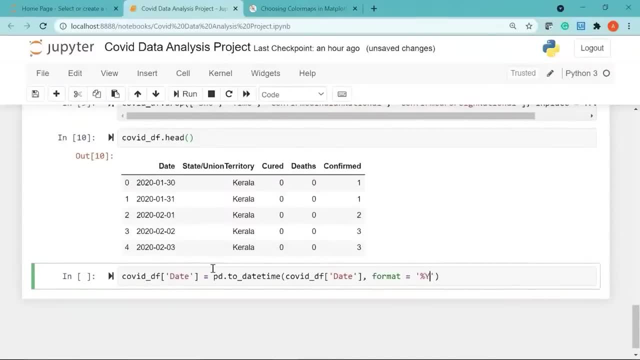 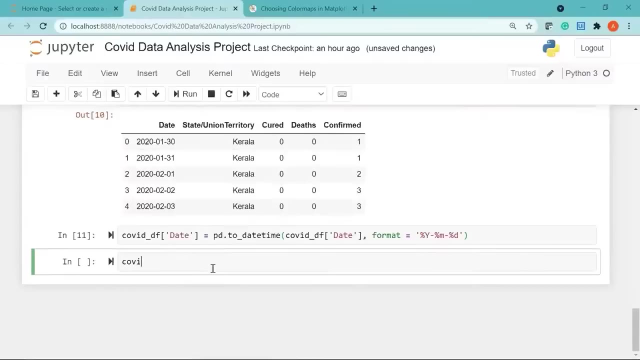 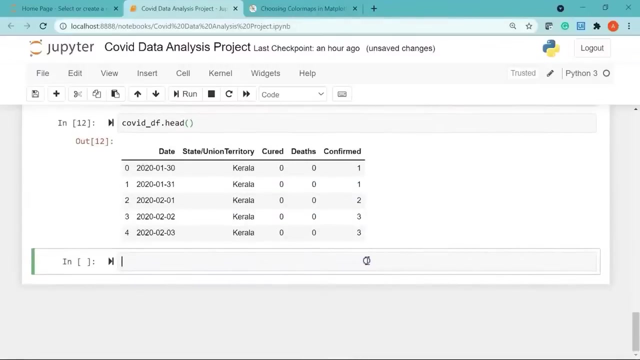 equal to. i'll say percentage y, give a dash, say percentage m, give another dash and say percentage d. let's run it and i'll print the head of the data frame. cool, now moving ahead. now we will see how to find the total number of active cases. 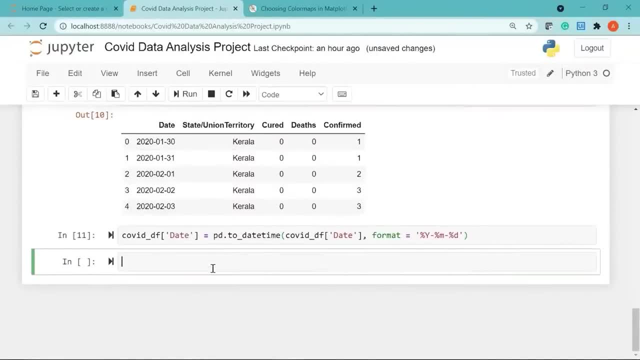 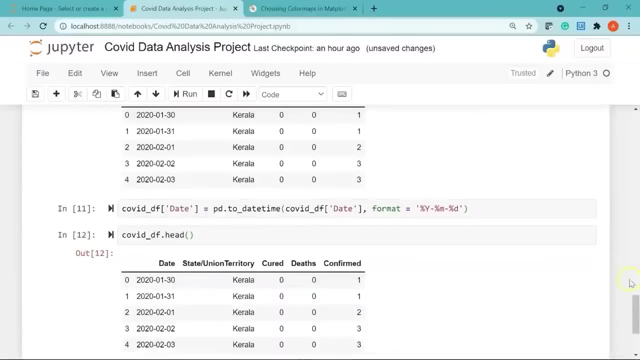 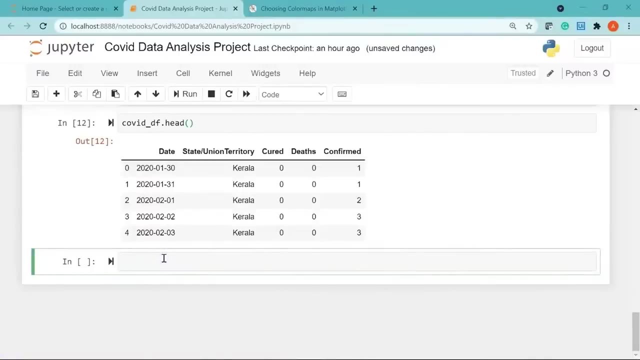 d. let's run it and i will print the head of the data frame. cool, now moving ahead. now we will see how to find the total number of active cases. so active case is nothing but the total number of confirmed cases minus the sum of cured cases plus. 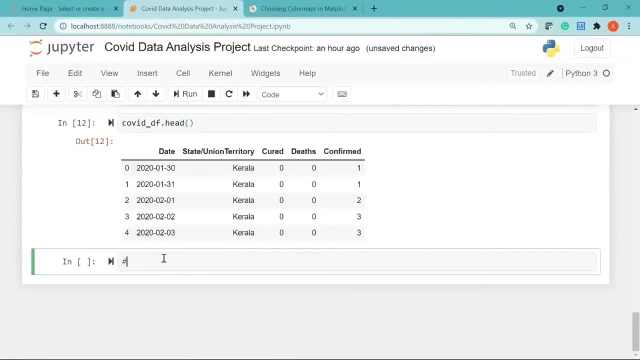 deaths reported. so let's find the active cases and i will give a comment. ok, i will first write my data frame name, that is covid underscore df. within square brackets. i will give my new column, which is active underscore cases. i will say: equal to covid underscore df. 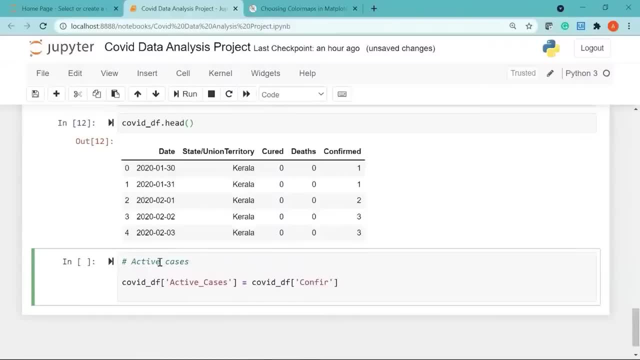 and my first column would be the confirmed cases column minus. i will say covid underscore df, then i will pass in my cured column plus. i will again say covid underscore df and add my deaths column. this time let's print the last five rows from the new data frame. 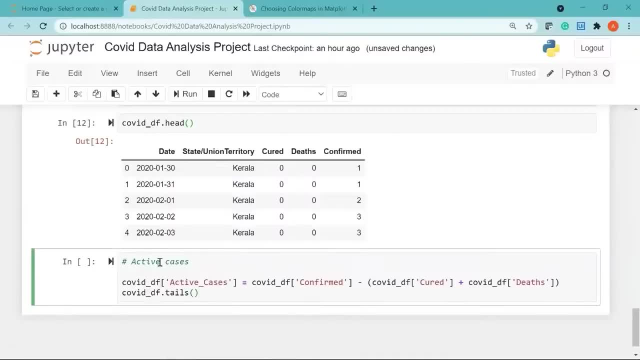 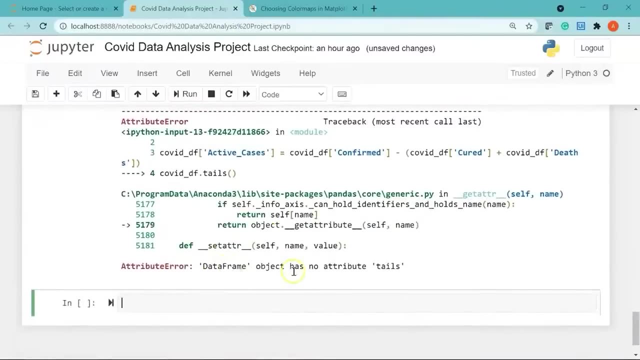 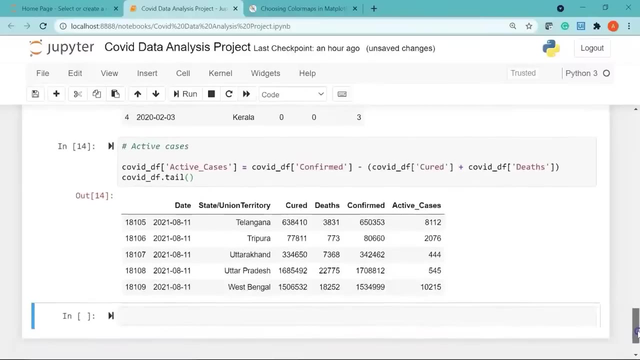 that we have created. ok, let's run it. it has thrown an error. let's debug. it says data frame object has no attribute tails. this should be tail. there you go, you can see here we have added a new column called active cases, which is the confirmed cases minus the sum of 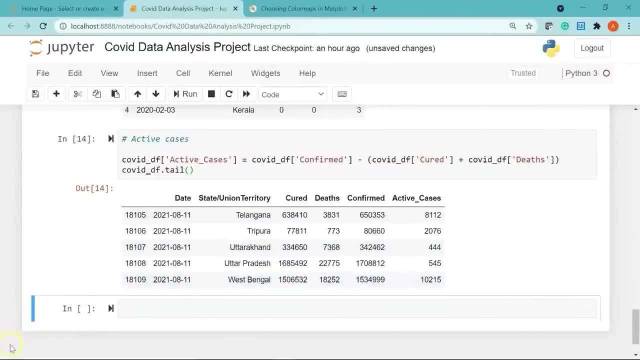 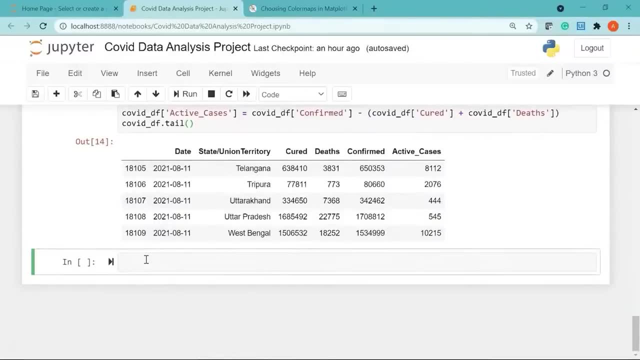 cured and deaths reported column. now we will learn how to create a pivot table using the pandas library. so in this table we will be summing all the confirmed deaths and cured cases for each of the states and union territories. so we will be using the pivot underscore table function for 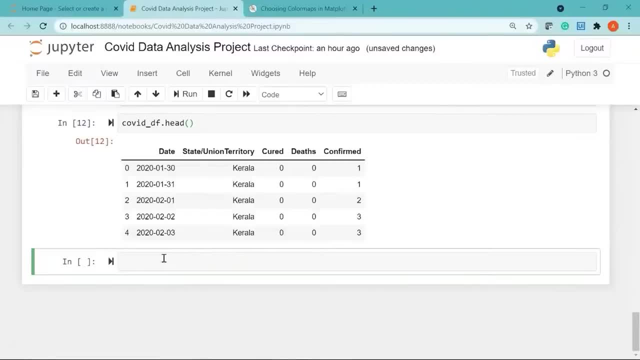 so active case is nothing but the total number of confirmed cases minus the sum of cured cases plus deaths reported. so let's find the active cases. i'll give a comment. okay, i'll first write my data frame name, that is covid, underscore df, within square brackets. i'll give my new. 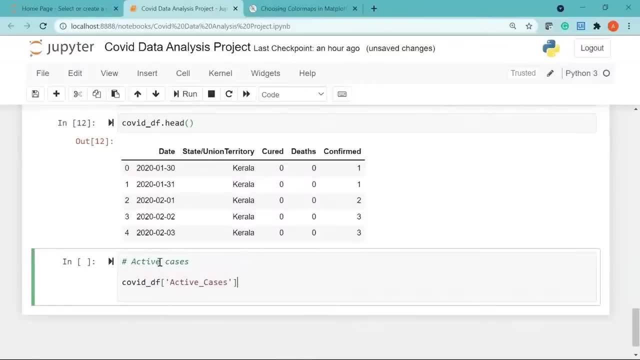 column which is active underscore df, which is active underscore cases, i'll say equal to covid underscore df and my first column would be the confirmed cases. column minus, i'll say covid underscore df. then i'll pass in my cured column plus, i'll again say covid underscore df. 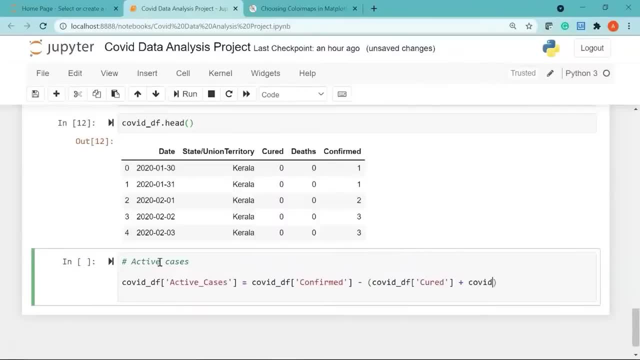 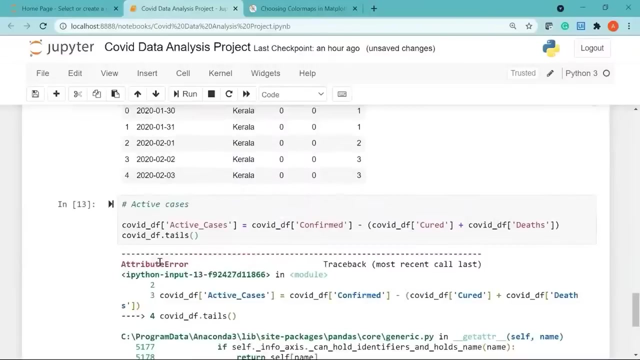 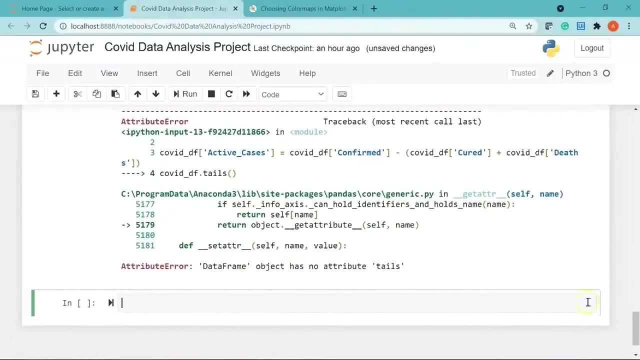 COVID, underscore DF and add my deaths column. this time. let's print the last five rows from the new data frame that we have created. okay, let's run it. it has thrown an error. let's debug. it says: data frame object has no attribute tails. this should be tail. there you go, you. 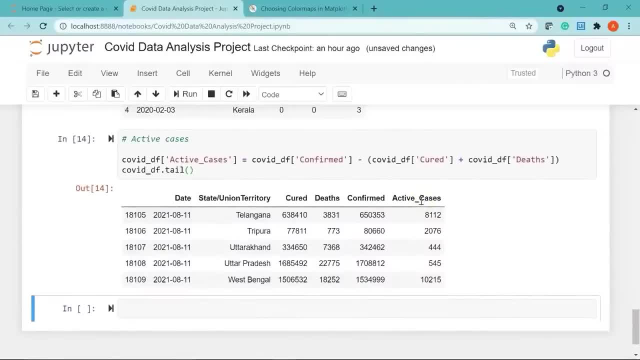 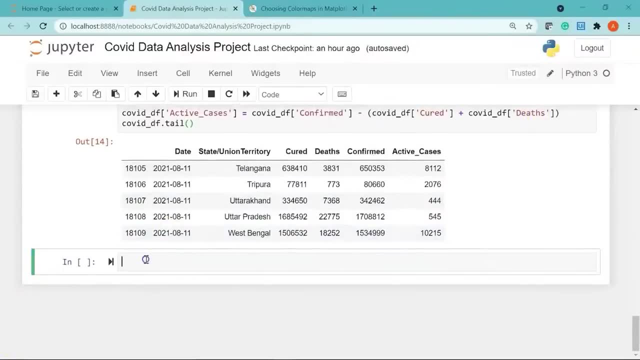 can see here we have added a new column called active cases, which is the confirmed cases minus the sum of cured and deaths reported column. now we will learn how to create a pivot table using the pandas library. so in this table we will be summing all the 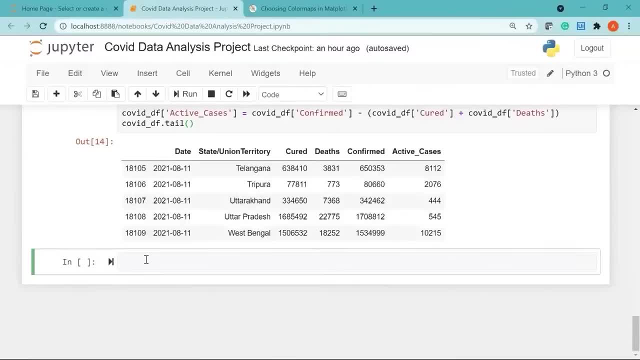 confirmed deaths and cured cases for each of the states and Union territories. so we'll be using the pivot underscore table function for this. I'll create a variable called statewide and say PD dot. I'll use the pivot underscore table function. I will pass in my data frame. 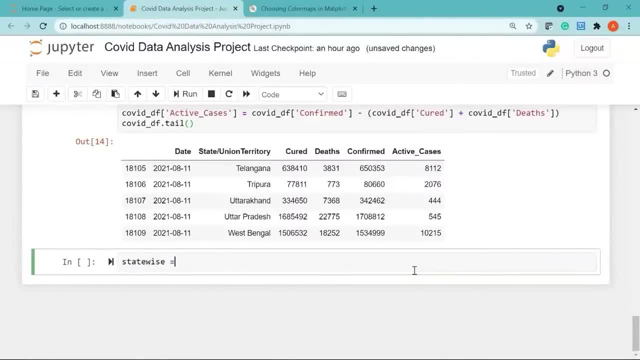 this. i will create a variable called state wise and say pd dot. i will use the pivot underscore table function. i will pass in my data frame that is covid underscore df, and then i will give my values parameter inside the square brackets i will pass in my columns. 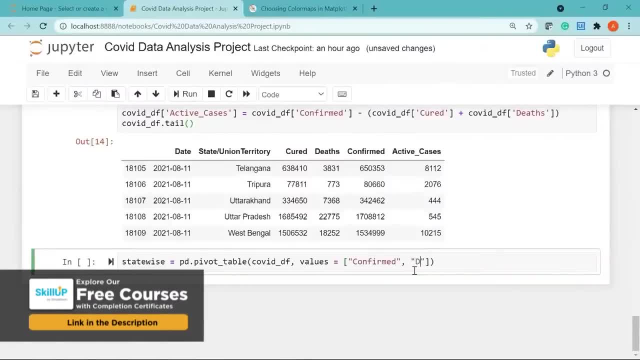 confirmed deaths. and then we will have the cured column: give a comma and next argument would be: index, which is going to be my state: slash the union territory column. let me bring this to the next line so it is more readable. i will say union territory, i will 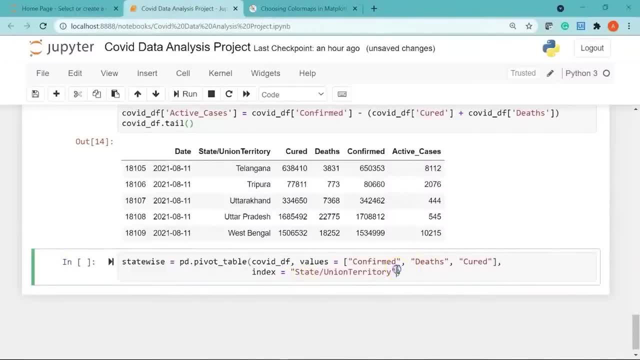 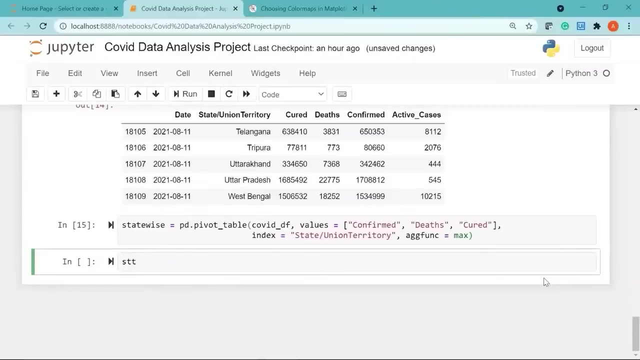 give a comma now and pass in my last argument, which is agg function. that means aggregate function and this function would be max. alright, let's run it now. i am going to find out the recovery rate. so recovery rate is basically the total number of cured cases divided by the total number of confirmed 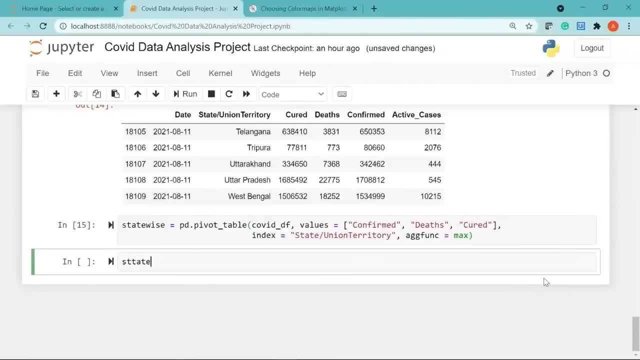 cases into 100. so i will say state wise and within square brackets, i will pass in my variable that i want to create, which is recovery rate. this will be equal to the cured cases multiplied by 100, by the total number of confirmed cases within square brackets. 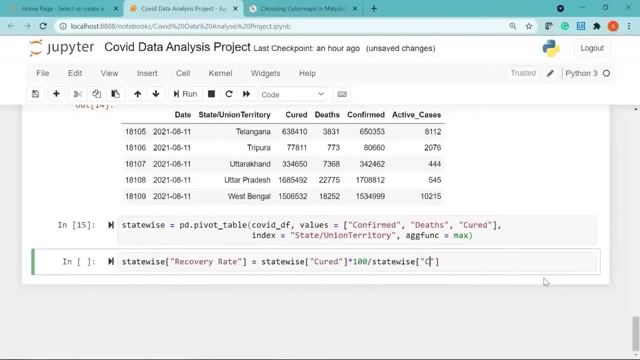 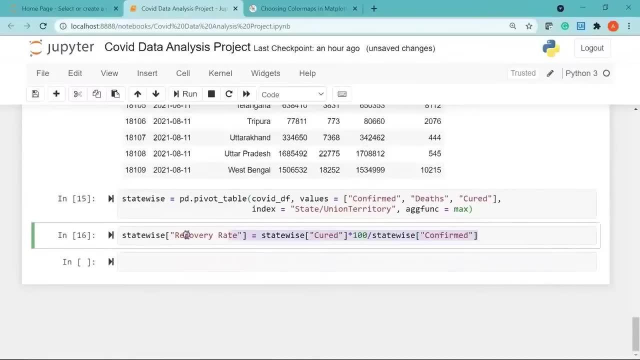 i will give my column as confirmed. let's run this. ok, i will just copy this column, paste it here. so this time we are going to find out the mortality rate. so mortality rate is nothing but the total number of deaths divided by the total number of confirmed cases into 100. 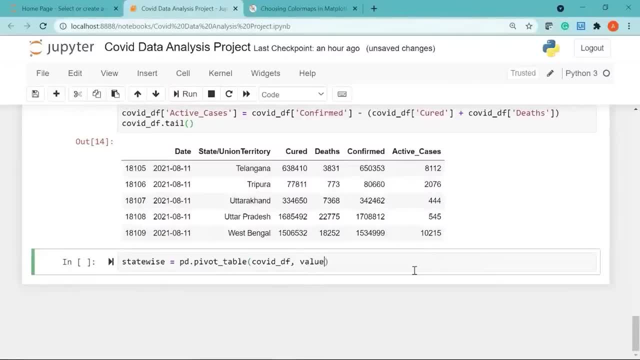 that is, COVID, underscore DF, and then we'll give my values parameter. inside the square brackets I'll pass in my columns confirmed deaths, then we'll have the cured column give a comma and next argument would be index, which is going to be my state slash the Union territory column. 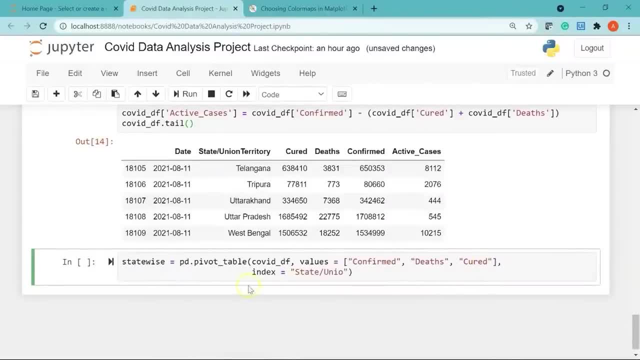 let me bring this to the next line so it is more readable. I'll say Union territory. I will give a comma now and pass in my data frame. so I will pass in my data frame and then I'll pass in my last argument, which is a GG function. that means aggregate function and this function. 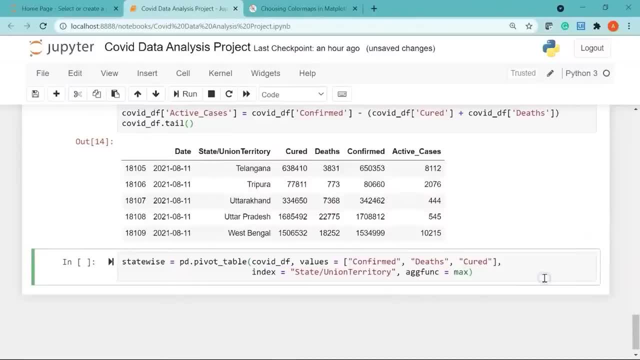 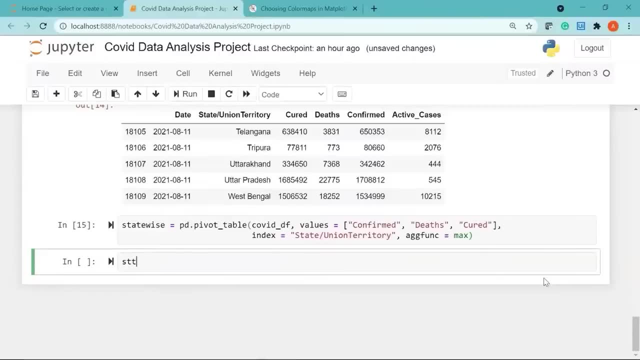 would be max. all right, let's run it. okay, now I'm going to find out the recovery rate. so recovery rate is basically the total number of cured cases divided by the total number of confirmed cases into 100. so I'll say state wise and within square brackets. 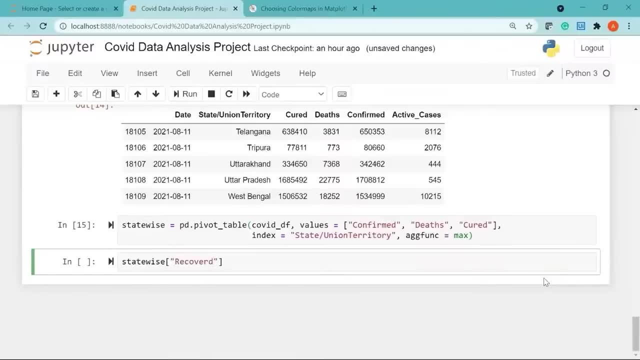 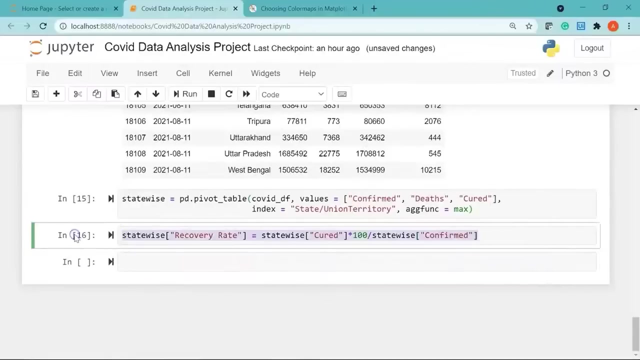 I'll pass in my variable that I want to create, which is recovery rate. this will be equal to the cured cases multiplied by 100, by the total number of confirmed cases within square brackets. I'll give my column as confirmed. let's run this okay, I'll just copy this column. 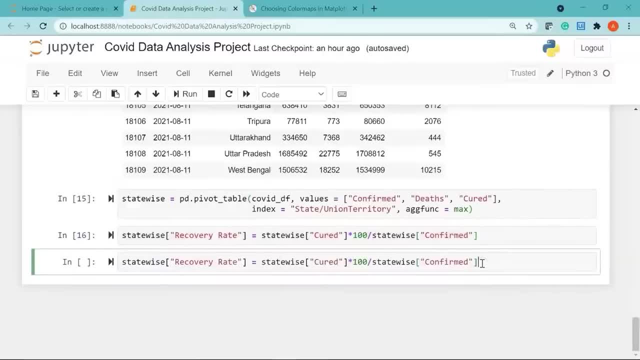 paste it here. so this time we are going to find out the mortality rate. so mortality rate is nothing but the total number of deaths divided by the total number of confirmed cases into 100. so I am just going to replace the names here. I'll say mortality, all right, and then instead of cured I'll say my deaths. 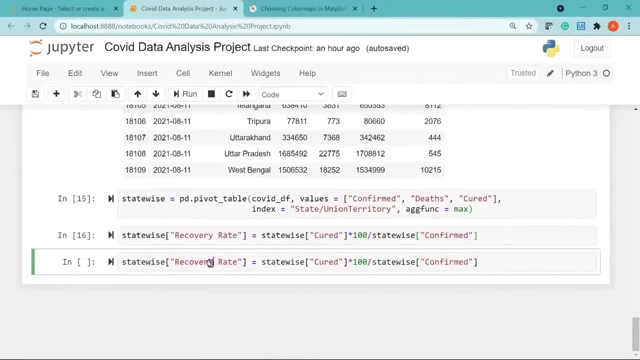 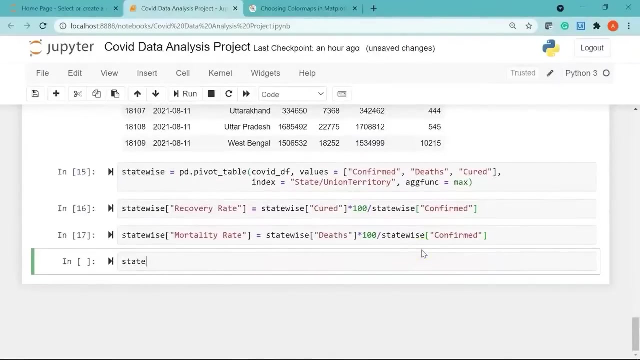 so i am just going to replace the names here. i will say mortality, alright, and then instead of cured i will say my deaths column into 100 divided by the confirmed cases. let's run it ok. now we are going to sort the values based on the confirmed cases column. 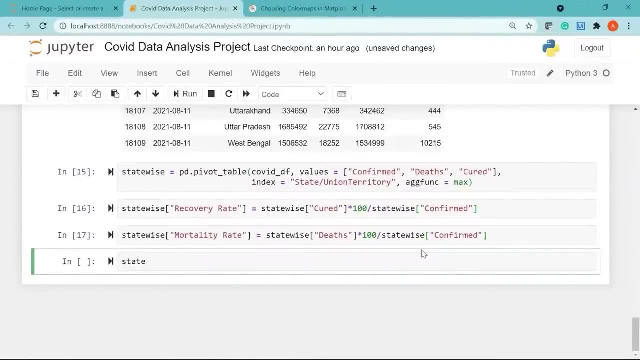 and we will sort it in descending order. so let me show you how to do it. i will say: state wise equal to. i will use the function sort underscore values. so i will pass in my variable state wise dot and use the short underscore values function. i will say: 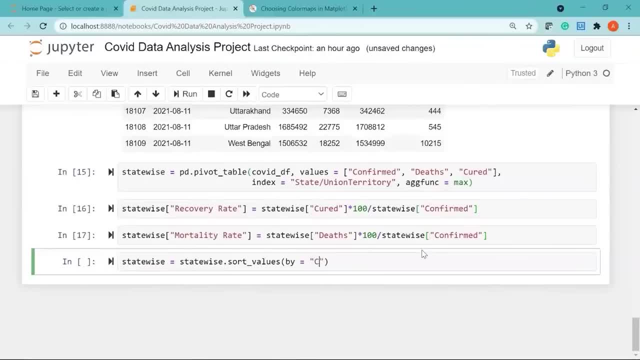 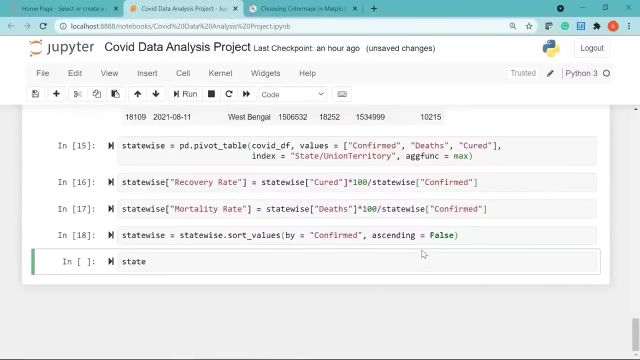 by. i want to sort it by my confirmed cases column. give a comma and i will say: ascending equal to false. let's run it now. we are going to plot our pivot table using a nice visual, so for that i am going to use my background underscore gradient. 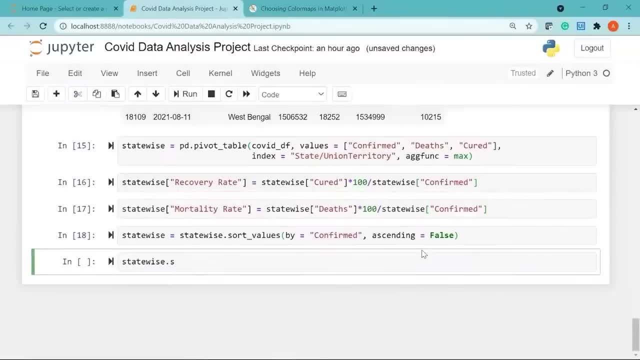 function and inside that function we will pass in our cmap parameter. i will show you how to do it. i will say style dot, background, underscore gradient, underscore gradient. and inside this we will pass in a parameter called cmap. so cmap stands for color maps. this is present inside. 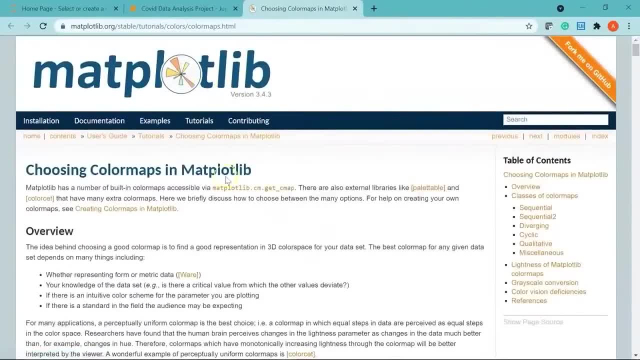 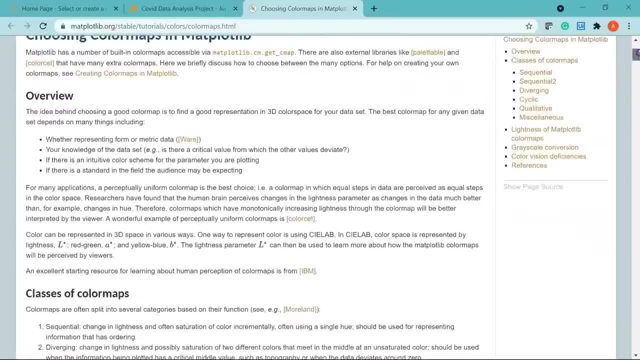 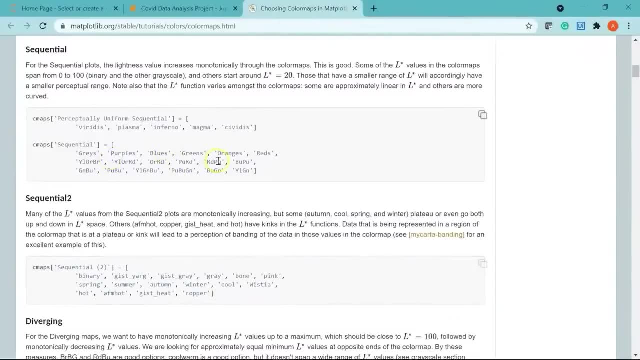 the matplotlib library. so here you can see there is a nice documentation on choosing color maps in matplotlib. this is provided by matplotlib dot org. if i scroll down you can see there are a number of cmaps that you can use. purples blues- you have something. 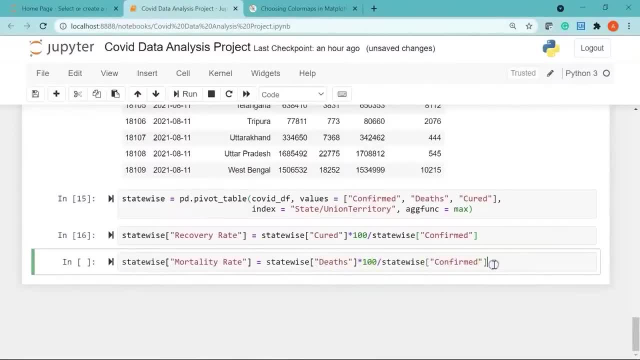 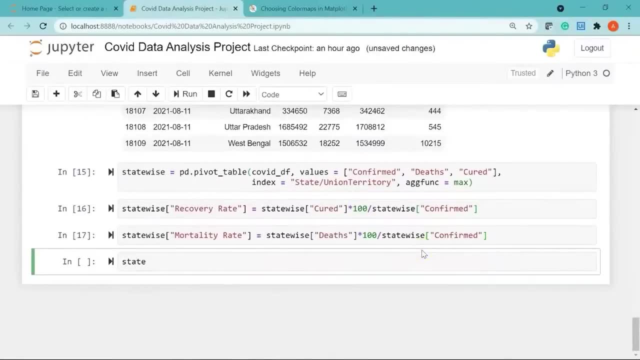 column into 100, divided by the total number of confirmed cases, into 100 ci lines to return deaths, and I'll say that my short underscore values function. I will say by: I want to sort it by my confirmed cases column, give a comma and I will say: 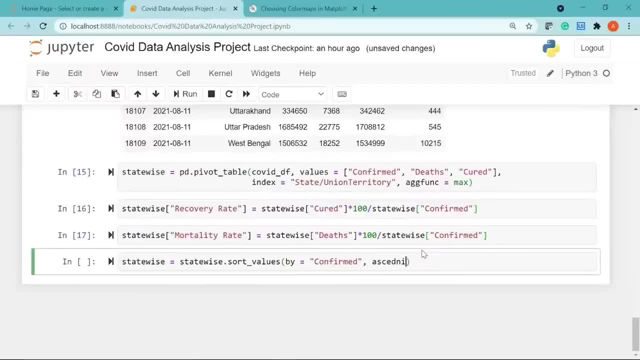 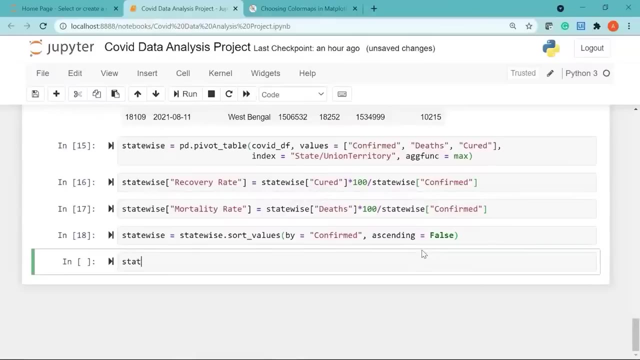 ascending equal to false. let's run it now. we are going to plot our pivot table using a nice visual, so for that I am going to use my background underscore gradient function and inside that function we will pass in our cmap parameter. I will show you how to do it. 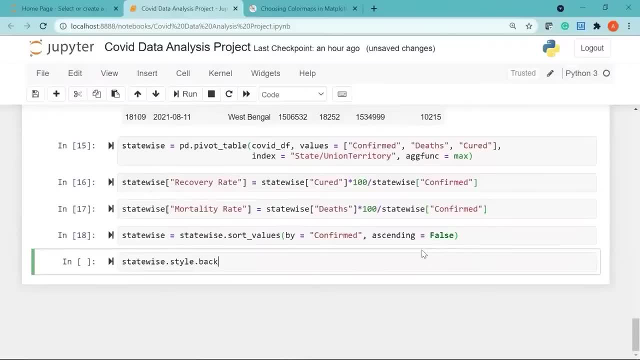 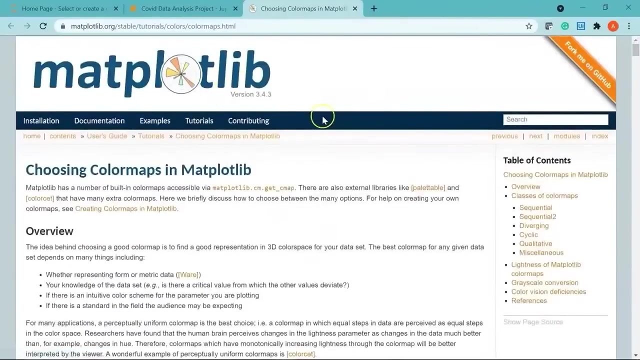 I will say style dot, background, underscore, gradient, and inside this we will pass in a parameter called cmap. so cmap stands for color maps. this is present inside the matplotlib library. so here you can see there is a nice documentation on choosing color maps in matplotlib. this is provided by matplotlib dot org. 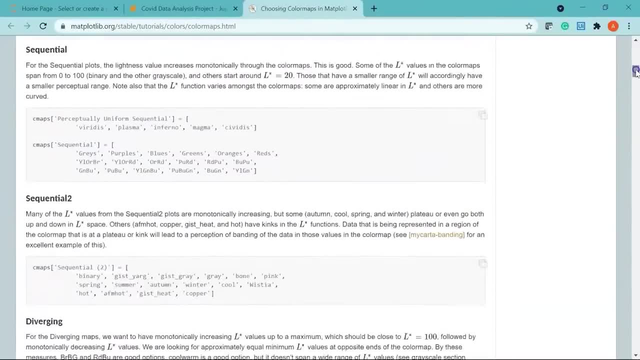 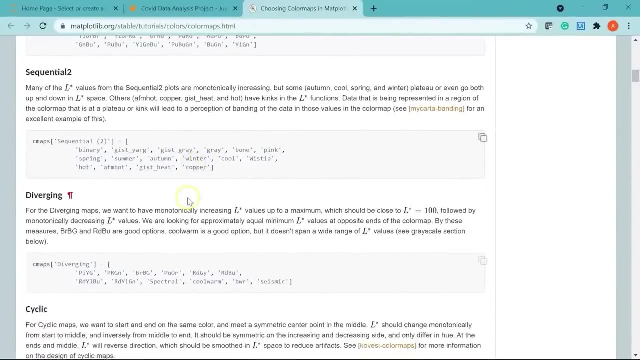 if I scroll down, you can see there are a number of cmaps that you can use: purples, blues. you have something called reds. there are other things like magma. you have summer, autumn, spring, winter, cool. all these you can use whichever color map that you want and here you can. 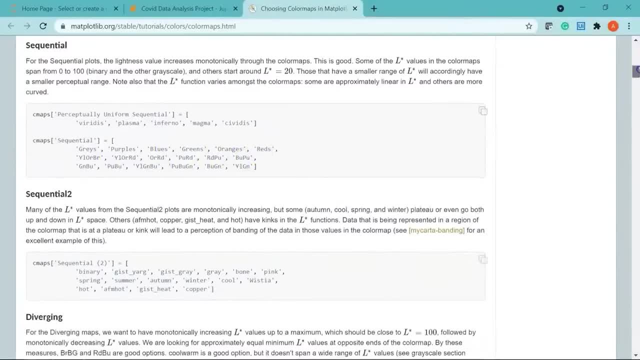 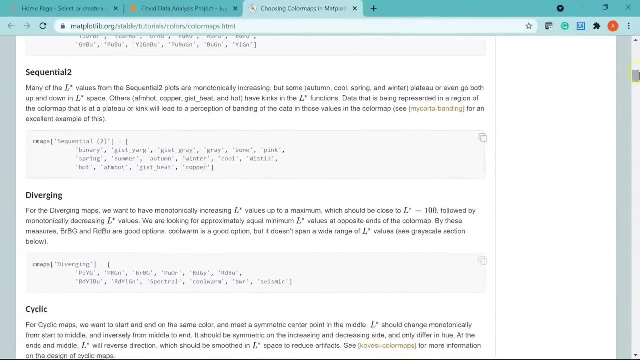 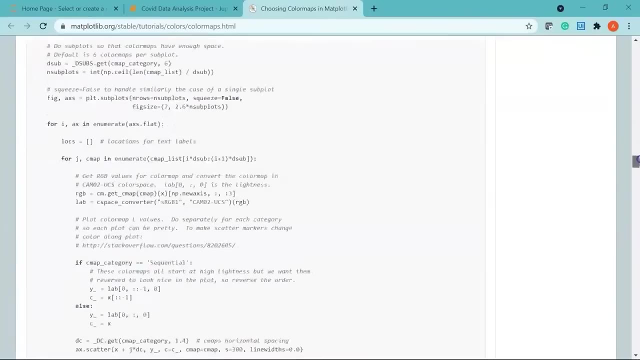 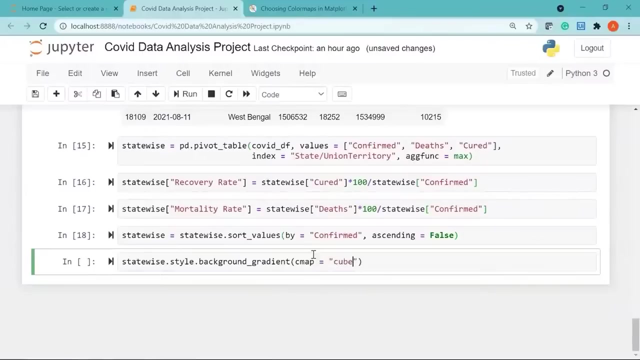 called reds. there are other things like magma. you have summer, autumn, spring, winter, cool. all these. you can use whichever color map that you want, and here you can see the different shades or the gradients. ok, so i am going to use my color map as cube helix. 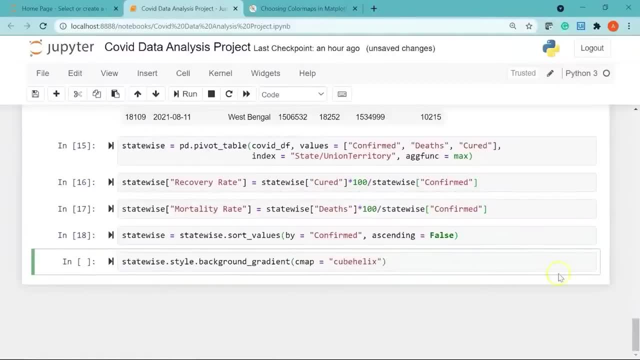 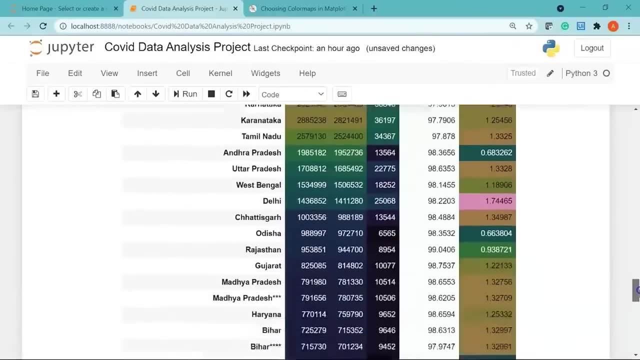 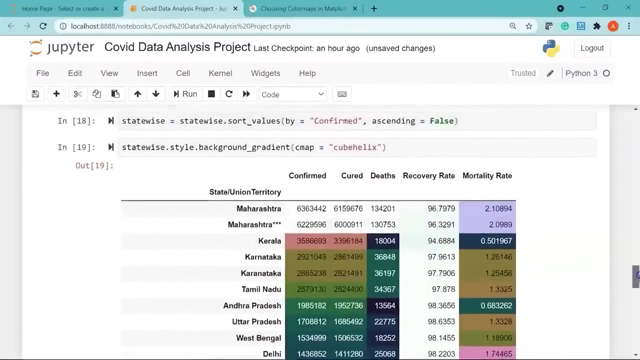 let me run it and show you the pivot table. there you go. here you can see. we have our pivot table ready now. as i said in the beginning, there are a few discrepancies in the data set, so here you can see. there is one called maharashtra. 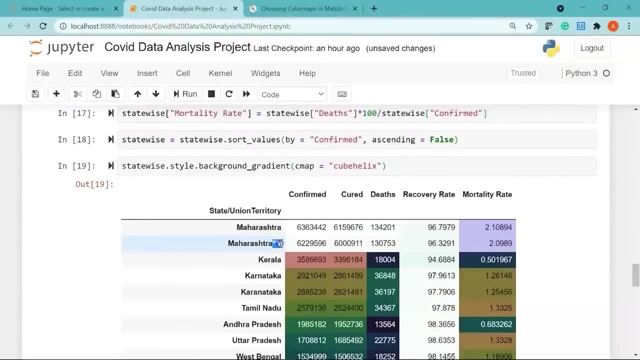 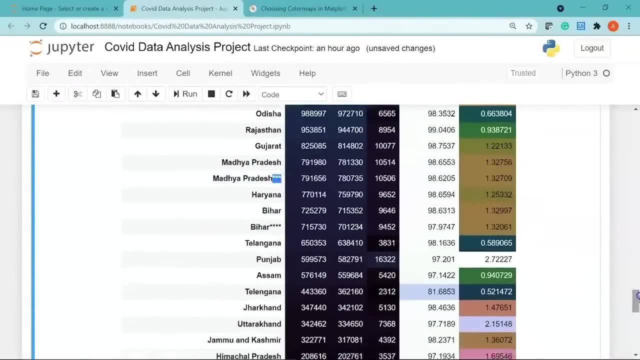 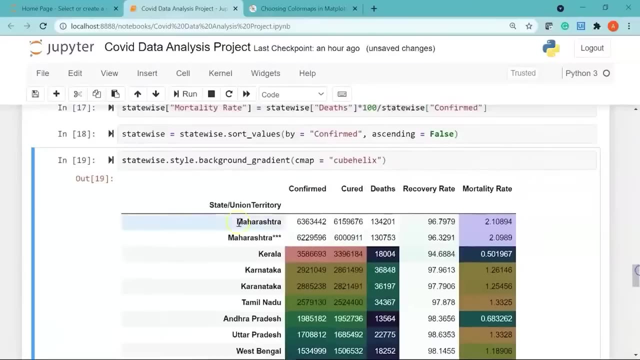 and there is also maharashtra triple star. this you can ignore. even if i scroll down, you have madhya pradesh followed by three asterisks. you can ignore this value as well. even for bihar we have. so these have been duplicated and here you can see the different. 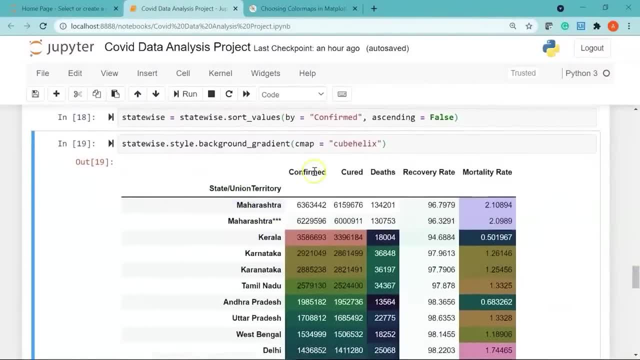 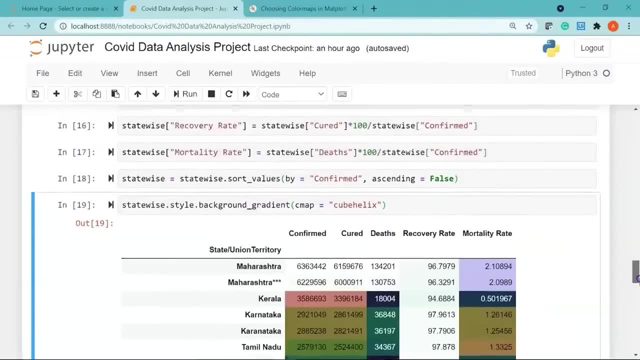 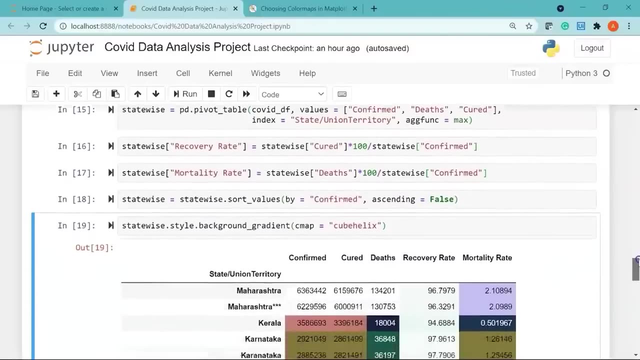 state names and union territories. then on the top you have the confirmed cases, cured cases, the deaths reported and the new columns that we created. these are calculated columns, recovery rate and mortality rate- and we have ordered it in december and this is the pending order of confirmed cases. 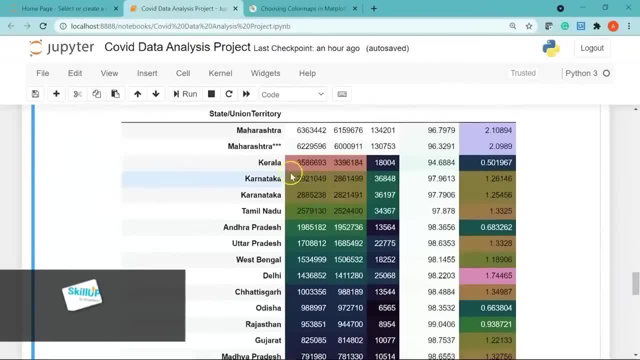 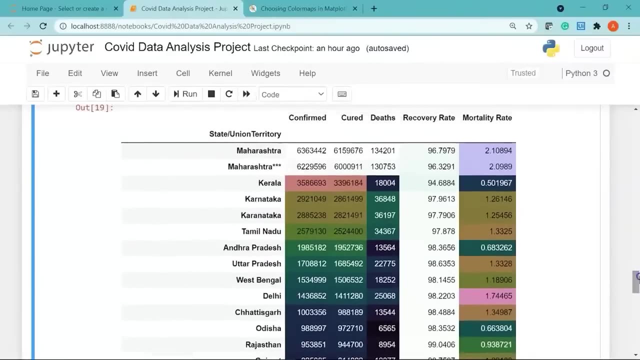 so so far, our data says that maharashtra has the highest number of cases, followed by kerala, karnataka, tamilnadu, andhra pradesh and uttar pradesh. so these are the top five states which have the highest number of confirmed cases, even if you see the mortality rate. 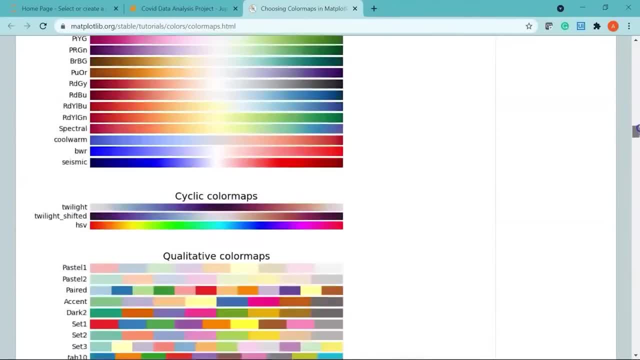 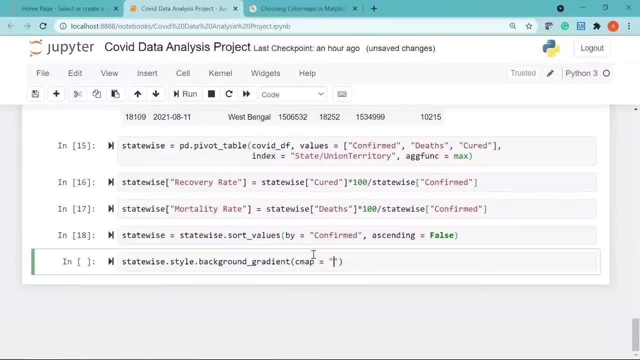 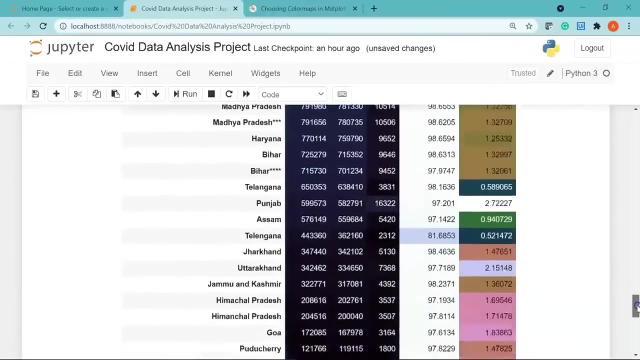 see the different shades or the gradients. okay, so I am going to use my color map as cube helix, let me run it and show you the pivot table. there you go. here you can see we have our pivot table ready now. as I said in the beginning, there are a few discrepancies. 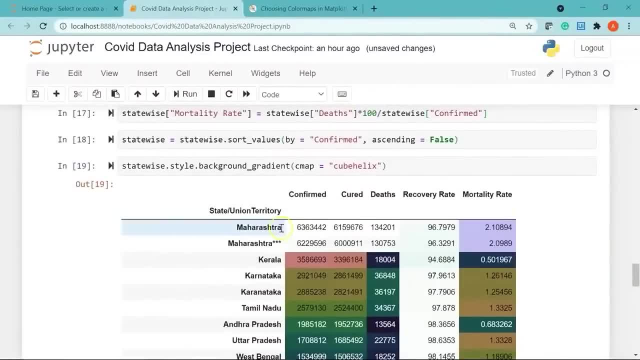 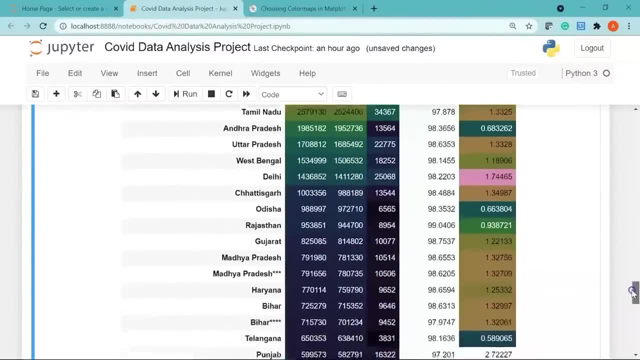 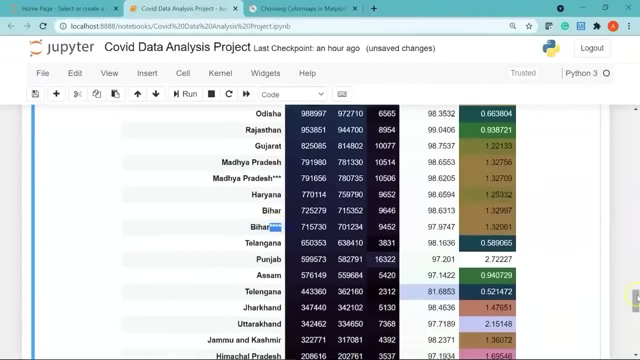 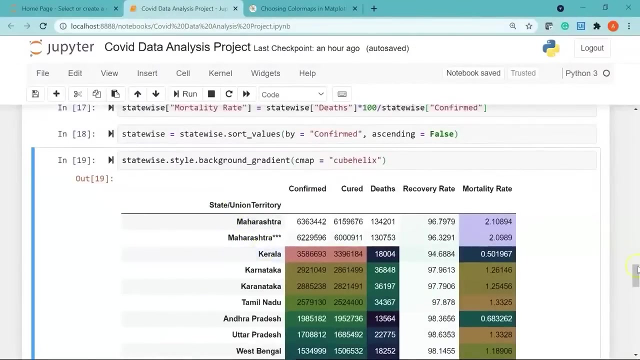 in the data set. so here you can see this one called Maharashtra, and there's also Maharashtra triple star. this you can ignore. even if I scroll down, you have Madhya Pradesh, followed by three asterisks. you can ignore this value as well, even for Bihar we have. so these have been duplicated and here you can see the different state. 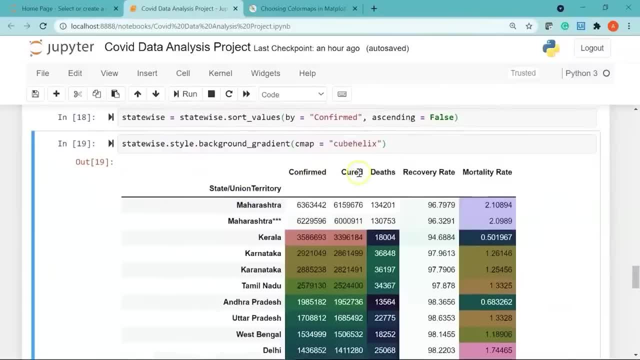 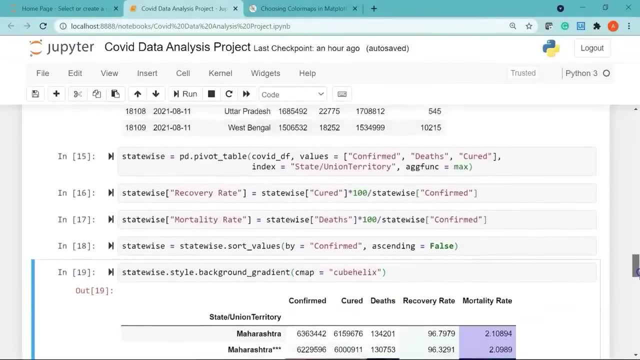 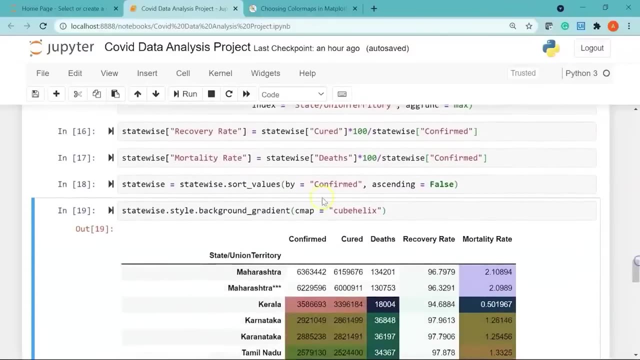 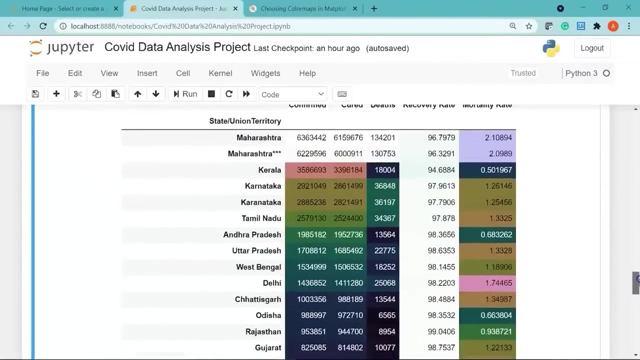 names and union territories. then on the top you have the confirmed cases, cured cases, the deaths reported and the new columns that we created. these are calculated columns- recovery rate and mortality rate- and we have ordered it in descending order of confirmed cases. so so far our data says that Maharashtra. 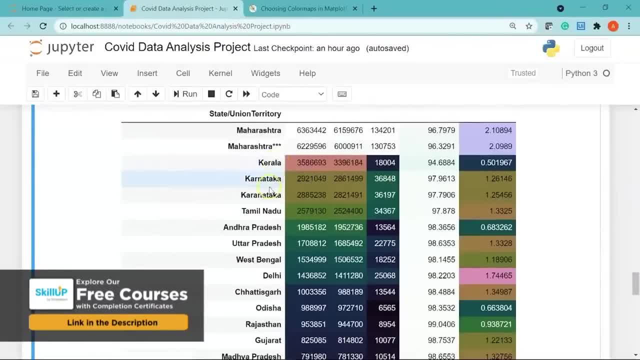 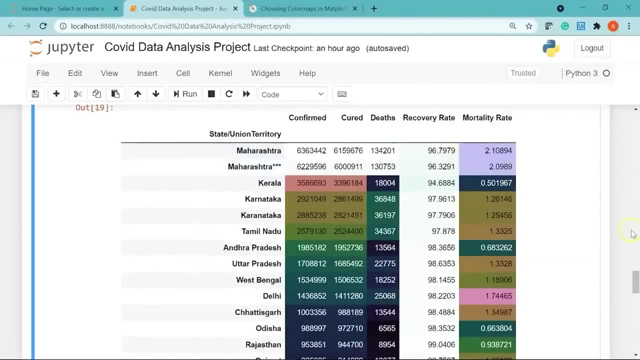 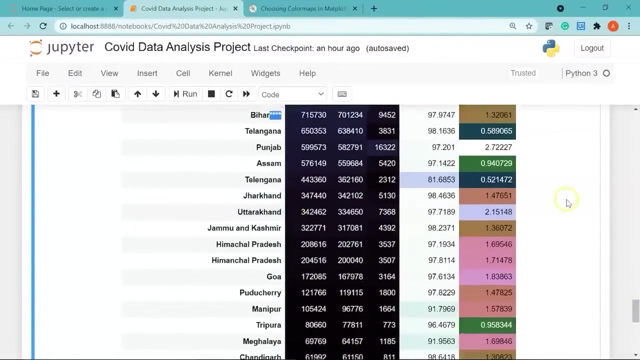 has the highest number of cases, followed by Kerala, Karnataka, Tamil Nadu, Andhra Pradesh and Uttar Pradesh. so these are the top five states which have the highest number of confirmed cases. even if you see, the mortality rate is also high for Maharashtra and if I scroll down, the mortality rate is also high for Uttarakhand, if you see here. 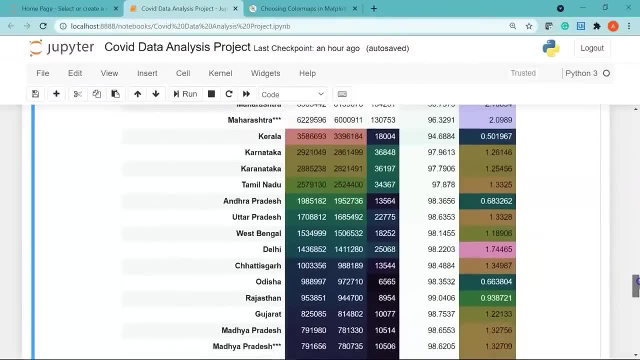 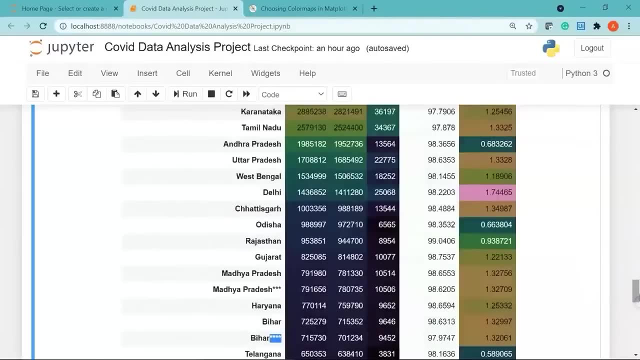 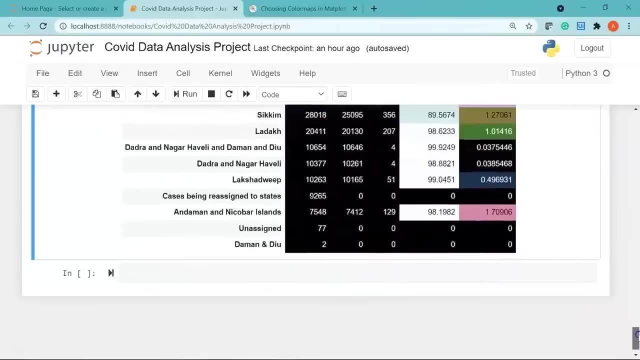 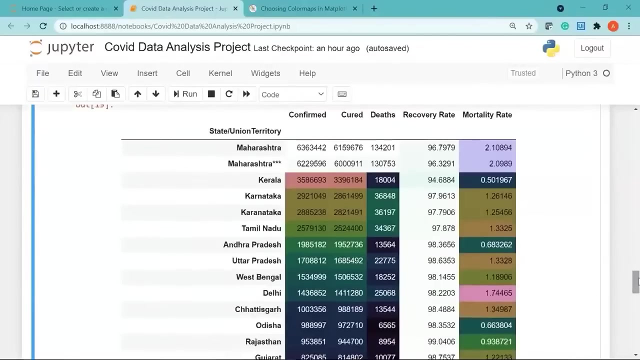 is also high for maharashtra and if i scroll down, the mortality rate is also high for uttarakhand. if you see here, if i scroll further, we have punjab. the mortality rate is also high. alright, so this was our first visual that we created in the 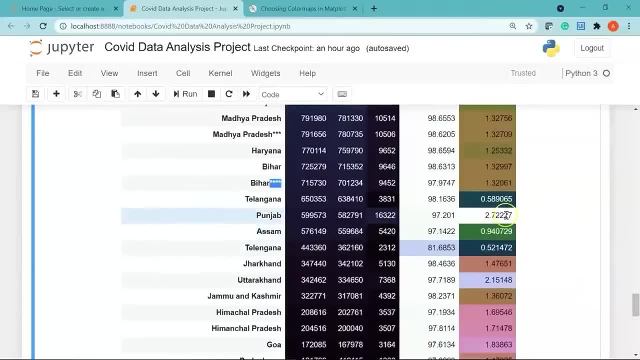 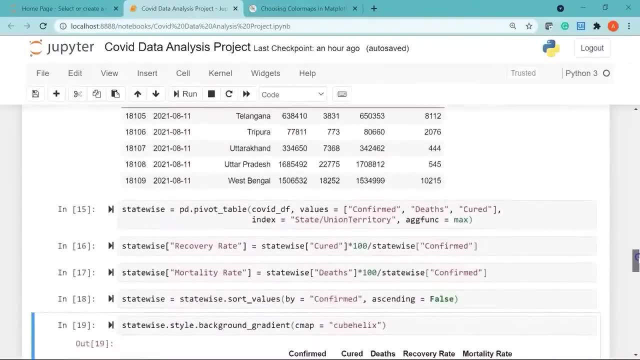 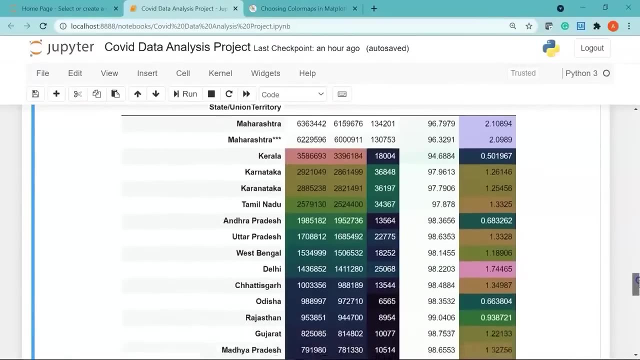 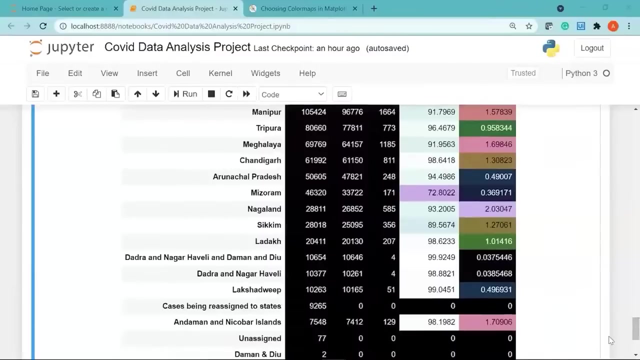 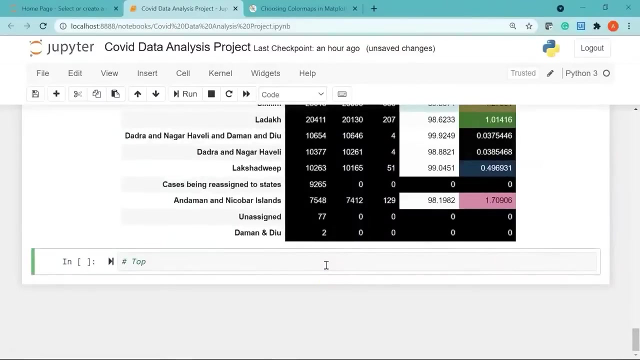 if I scroll further, we have Punjab. the mortality rate is also high. all right, so this was our first visual that we created in the COVID data analysis project. now, moving ahead, we'll see the top 10 states based on the number of active cases. so we will start. I'll give a comment. 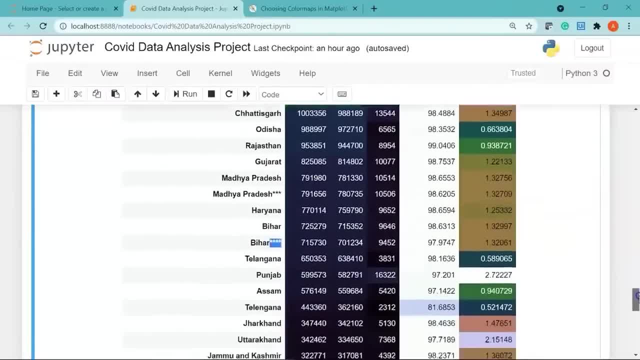 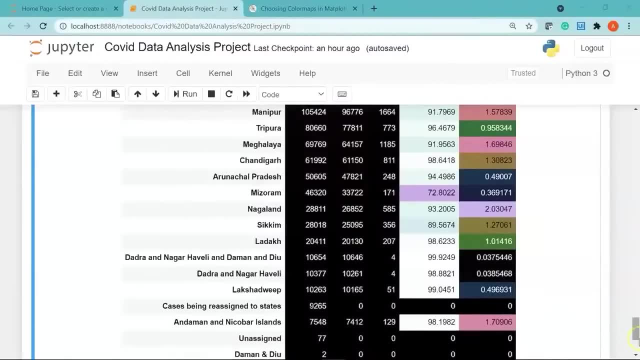 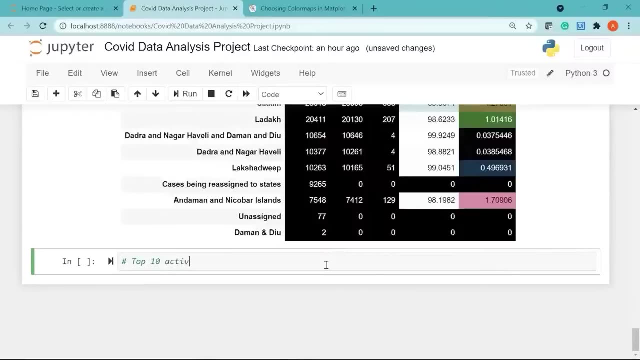 covid data analysis project now moving ahead. we will see the top ten states based on the number of active cases. so we will start. i will give a comment: top ten active cases states. ok, so we are going to explore another very important pandas function in this, which is known as. 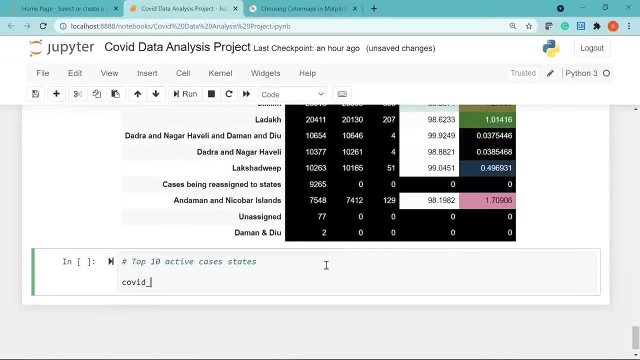 groupby. so i will first pass in my data frame, which is covid, underscore, df, dot, followed by the groupby function. i am going to group my data based on state slash union territory column. then i will say dot max, which is to find the maximum value from the states. 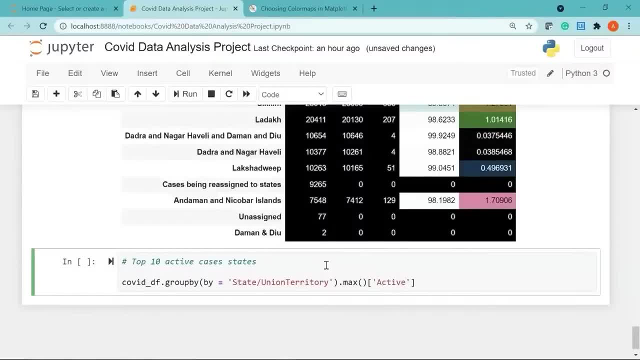 that have the highest active cases. so i have passed in my active cases column and we are also going to group it based on the date column. after that we are going to sort the values. so i will use my function that is sort underscore values. i will say: 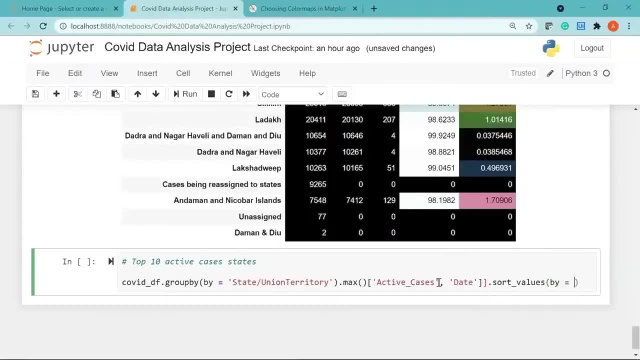 sort by my column, that is, active cases. let me bring this to the next line: underscore cases. i will give a comma and say ascending equal to false, say dot, and then i reset index. for that i will use reset underscore index function. ok, let's check if everything is fine. 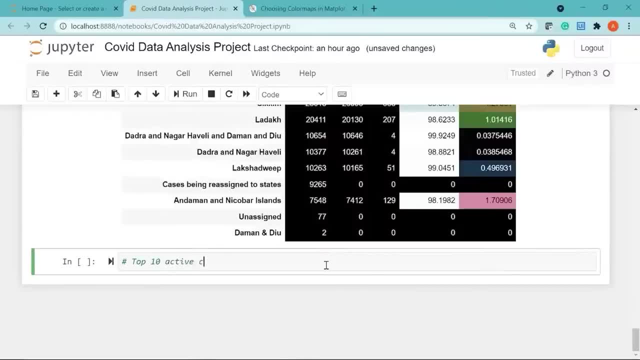 top 10 active cases states: okay, so we are going to explore another very important PANDAS function in this, which is known as group bye. so I'll first pass my data frame, which is COVID, underscore DF dot, followed by the group by function. I am going to group my data based on: 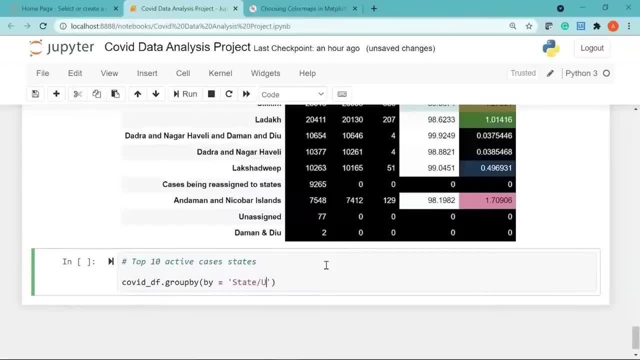 state slash union territory column. then I will say dot max, which is to find the maximum value from the states that have the highest active cases. so I have passed in my active cases column and we are also going to group it based on the date column. after that we are going to sort the values. so I will use my function. 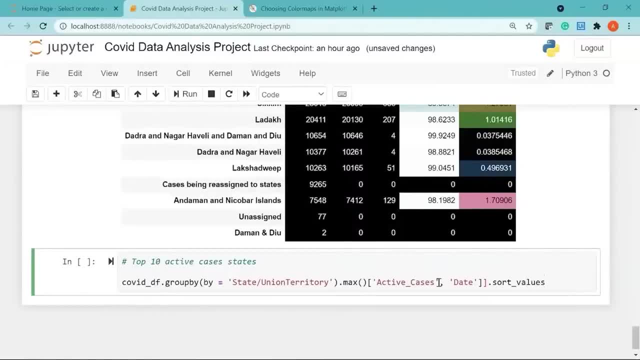 that is sort underscore values. I will say dot short by my column, that is active cases. let me bring this to the next line: underscore cases. I will give a comma and say ascending equal to false, say dot and then reset my index. for that I will use reset underscore index function. 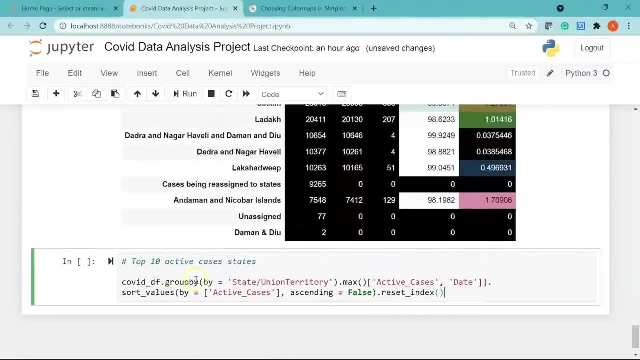 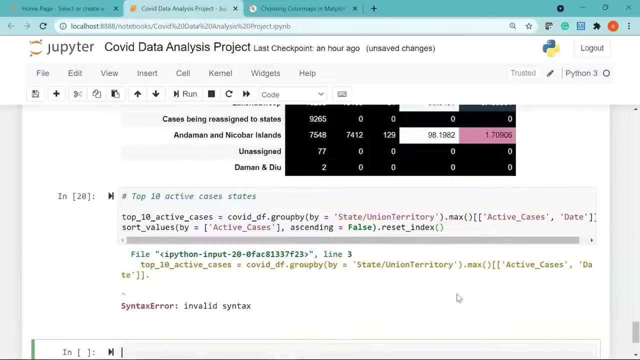 okay, let's check if everything is fine. I have missed a square bracket here. let me give another square bracket here. okay, and all this we are going to store in our variable called top underscore index. top underscore 10 underscore, active underscore cases. okay, now let me go ahead and run this cell. 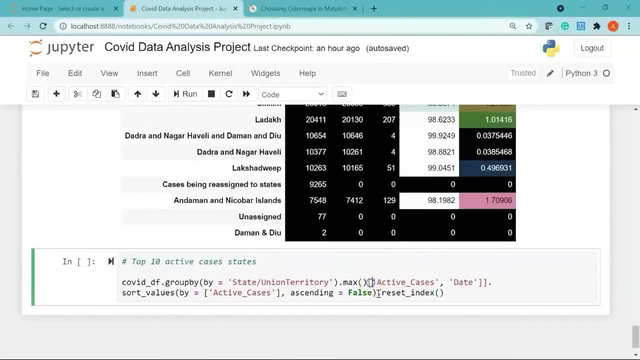 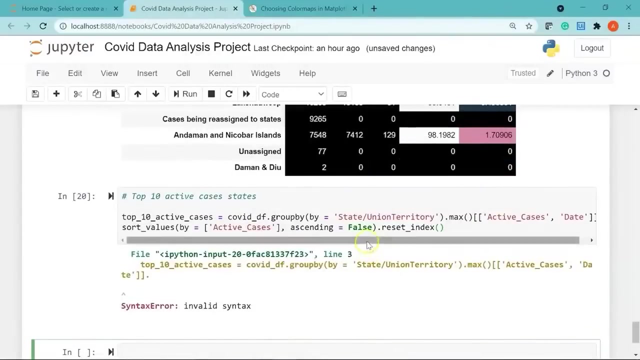 i have missed a square bracket here. let me give another square bracket here. ok, and all this we are going to store in our variable called top underscore, 10 underscore, active underscore cases. ok, now let me go ahead and run this cell. ok, there is a syntax error here. 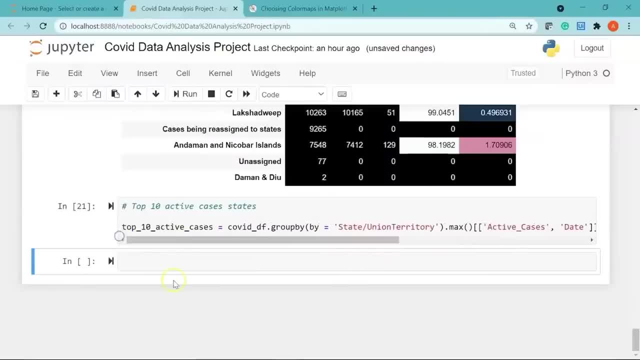 now let's run it. ok, now i will create another variable called fig. here we will pass in the plt, which is for matplotlib library, and we will give the figure size using the fig size argument equal to and within a tuple and passing the size, let's say 16. 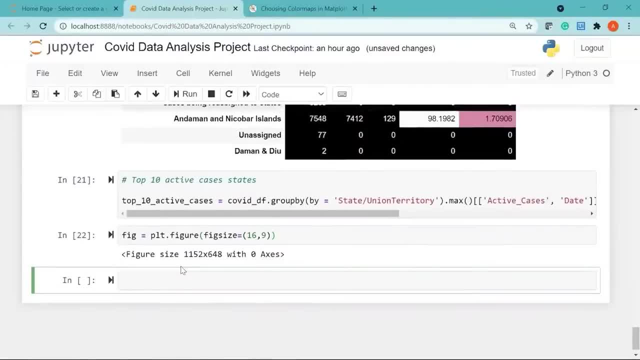 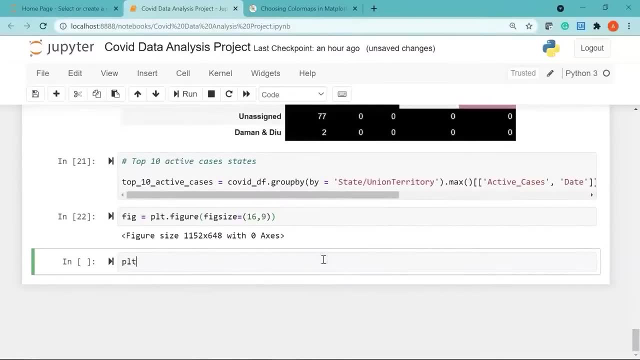 comma 9. we will run it ok, and let's give a title to our plot. so here we are going to create a bar plot. so using plt dot title, we will pass in the title. let's say top 10 states with most active cases in india. 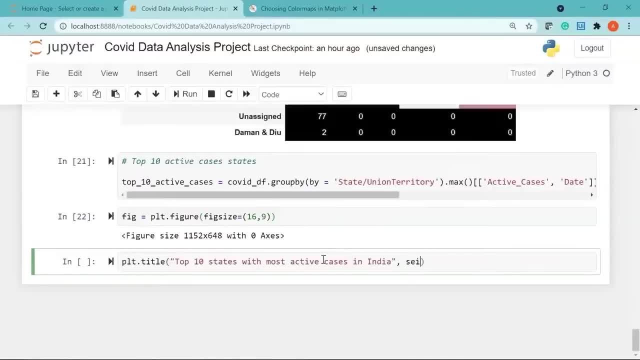 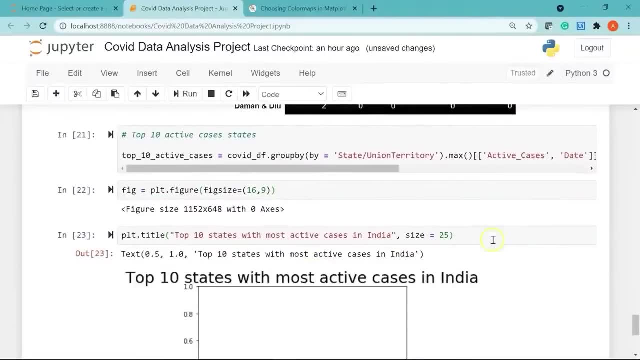 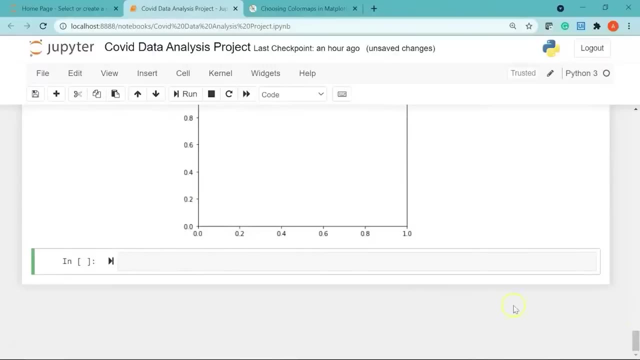 i will give a comma and pass in the size of my title, let's say 25. ok, you can see we are slowly being able to create our graph. the most important thing is to pass in the x axis and the y axis. i will say ax, which is for 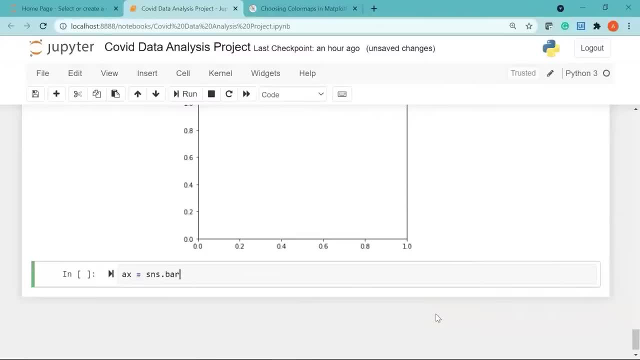 axis. to pass in the axis, i am going to use the barplot function that is present inside the seaborn library. i will say sns dot barplot. i will say data equal to my table, which is top underscore 10 underscore states. this is actually active states. alright, 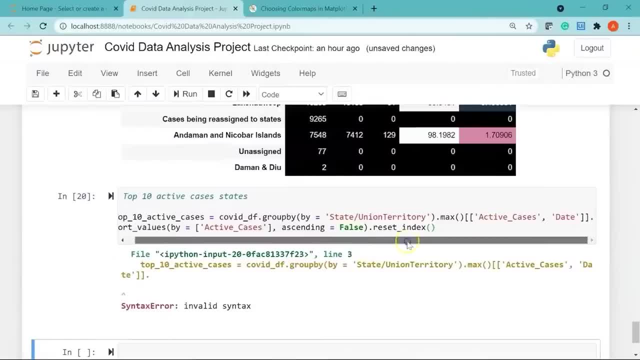 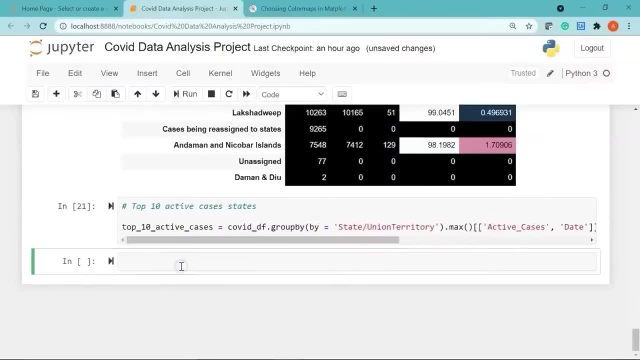 okay, there is a syntax error here. now let's run it. okay, now I will create another variable called fig. here we'll pass in the plt, which is for matplotlib library, and we'll give the figure size using the fig size argument is equal to and within a tuple, and passing the size, let's say 16 comma 9. 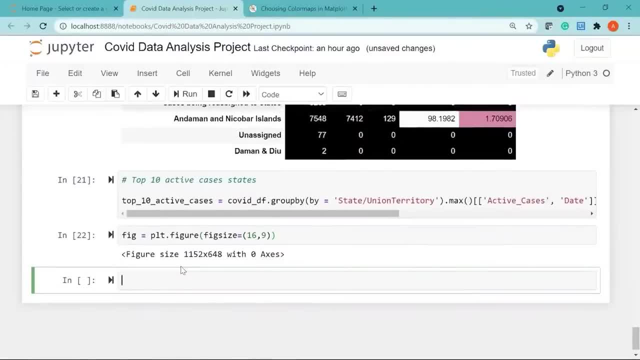 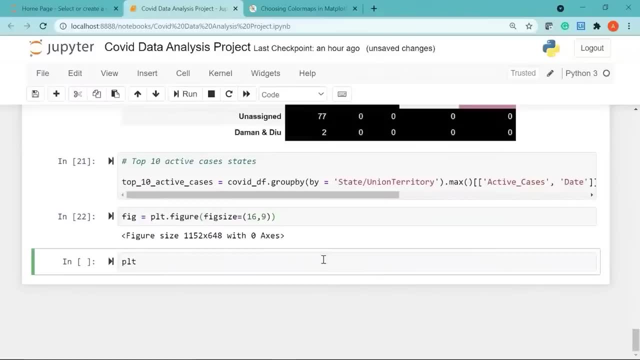 we'll run it okay and let's give a title to our plot. so here we are going to create a bar plot. so using plt, dot title will pass in the title. let's say top 10 states with most active cases in india. i'll give a comma and pass in the size of my title, let's say 25. 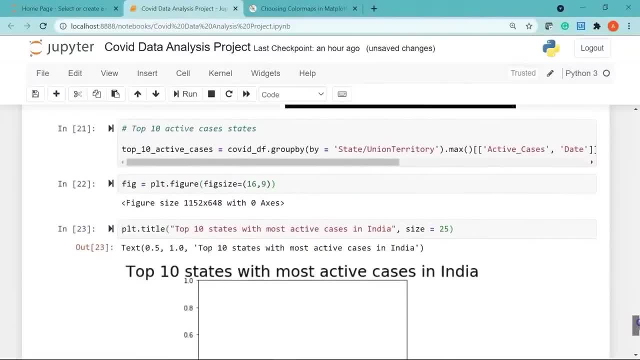 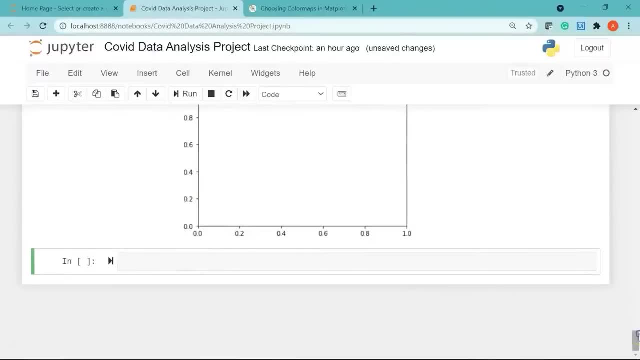 okay, you can see we are slowly being able to create our graph. the most important thing is to pass in the x-axis and the y-axis. i'll say ax, which is for axis to pass in the axis. i'll say ax, which is for axis to pass in the axis. i'll say ax, which is for axis. 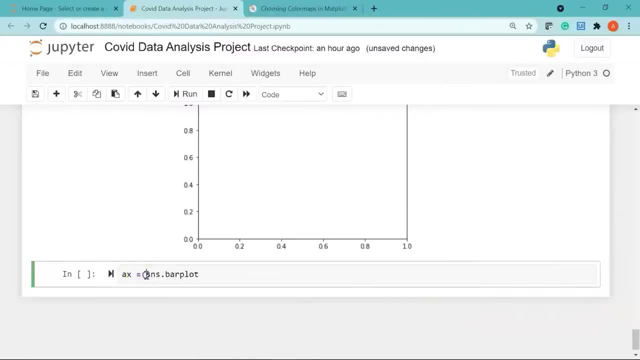 i'll say ax, which is for axis to pass in the axis. i'll say ax, which is for axis to pass in the axis, going to use the bar plot function that is present inside the seaborn library. i'll say snsbarplot. i'll say data equal to my variable, which is top underscore, 10 underscore states. 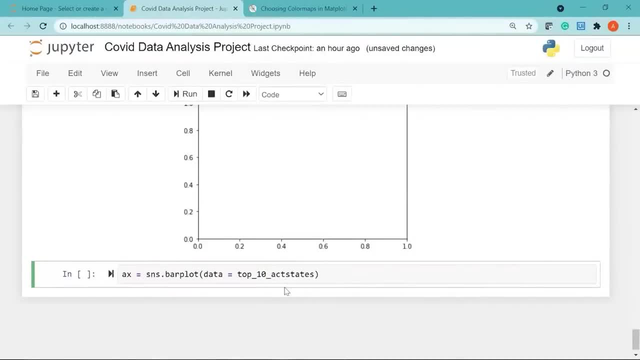 this is actually active states. all right, and now i'm going to use the iloc function and take the first 10 states. so i'm using a colon and then giving 10 as my value. iloc is for index location. i'll give a comma and say my y-axis to be: 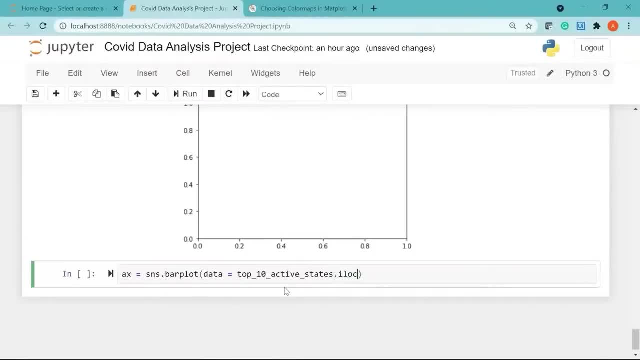 and now i am going to use the iloc function and take the first 10 states. so i am using a colon and then giving as my value iloc is for index location. give a comma and say my y axis to be active cases. give another comma. 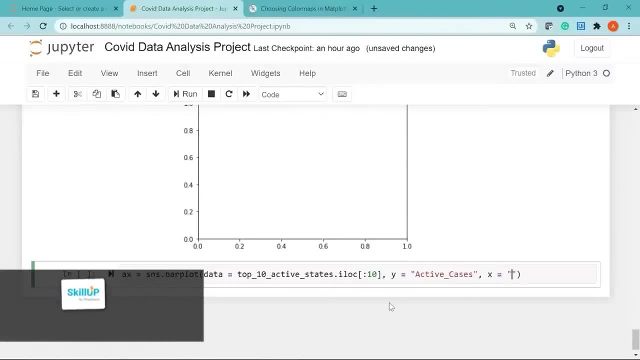 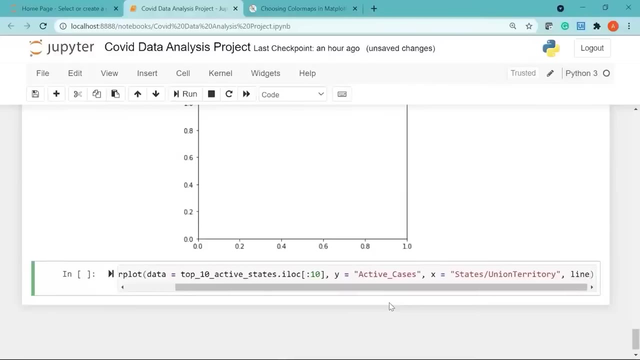 and say my x axis to be state slash union territory and say give another comma. we are going to pass in the line width to 2. i will say line width equal to 2 and will give an edge color. lets say the edge color is red. ok, 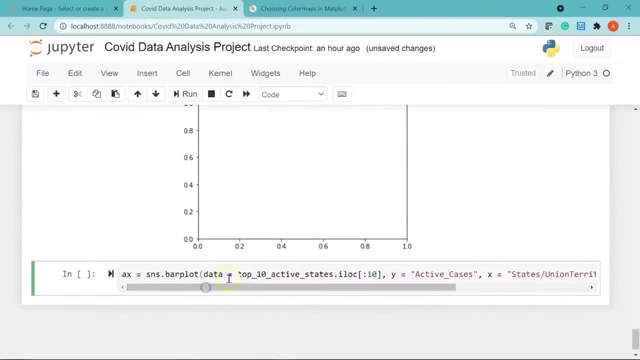 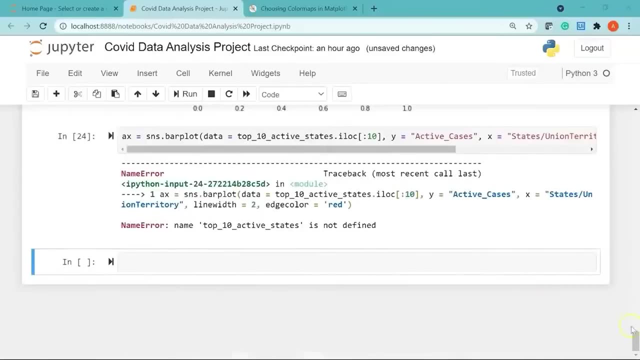 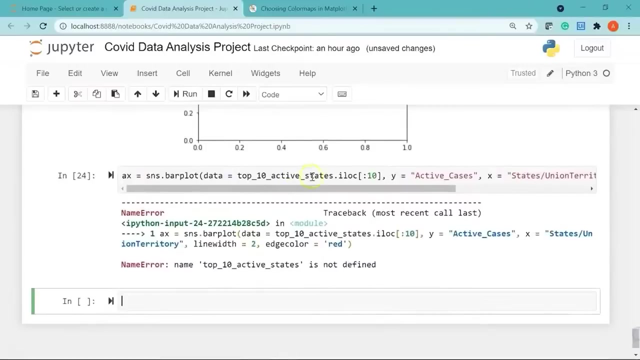 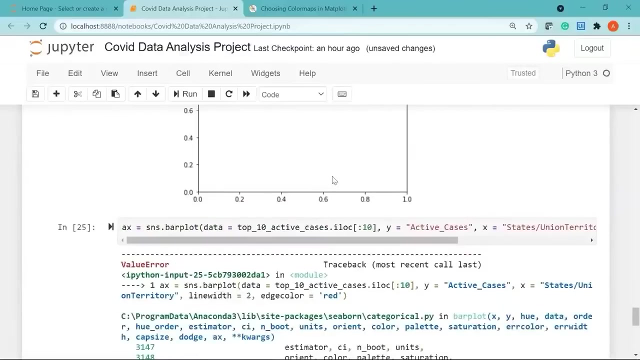 so i have my axis defined. now lets run it. there is an error here. it says: top 10 active states not found. lets go to the stop and see the exact. ok, so this is top 10 active cases. let me change it to cases here. now run it. 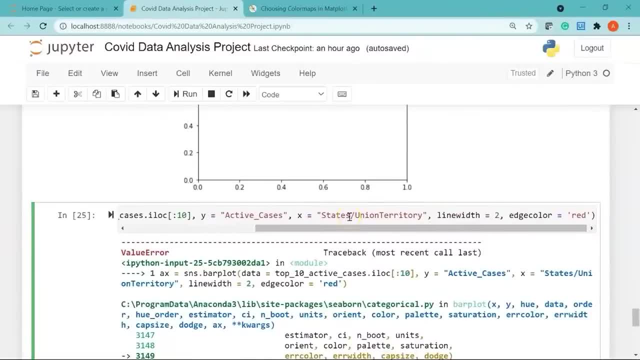 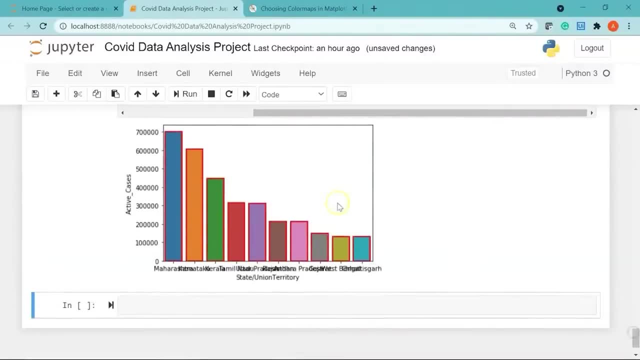 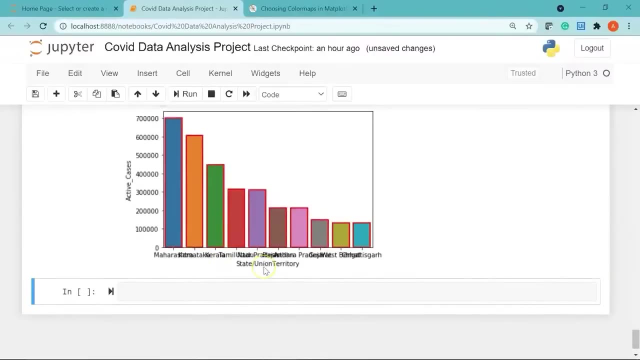 ok, the x axis also has a mistake. this should be state slash union territory. now let me run it. there you go. we have our plot created, but as you can see here, the labels of the different states and union territories are overlapping. so for that, let me first pass in the 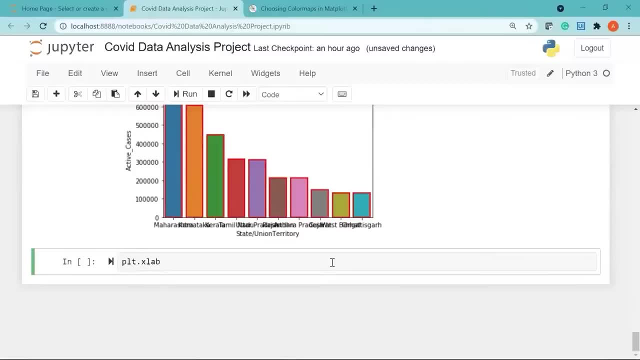 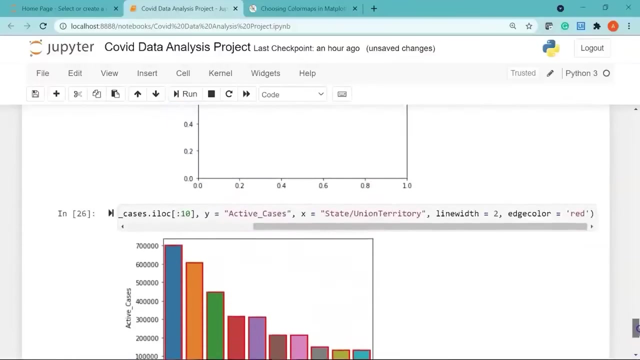 x labels. i will say plt dot x label and my x label would be states. then i will say plt dot y label. my y label will have the total active cases and finally i will write plt dot show. before i run it, lets collate all the lines of code that. 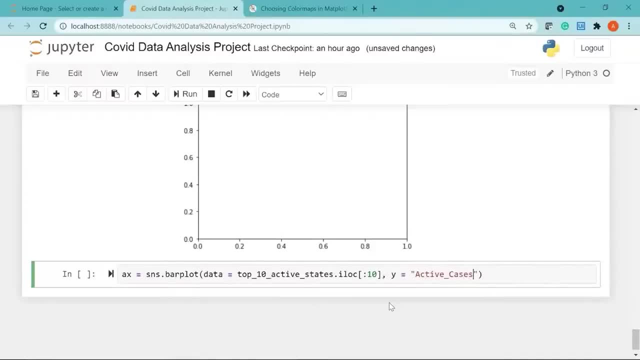 active cases. give another comma and say my x-axis to be state slash union territory. give another comma. we are going to pass in the line width to 2. i'll say line width equal to 2 and we'll give an edge color. let's say the edge color is red. okay, so i have my axis defined. now let's run it. 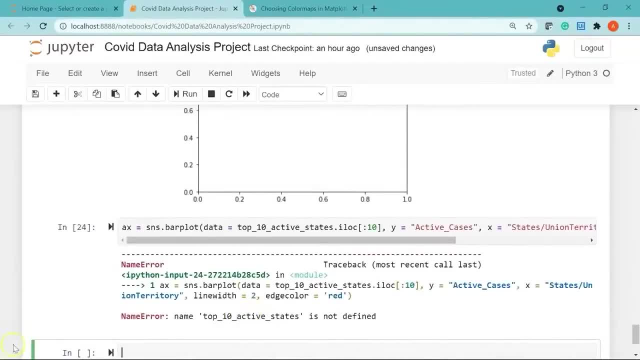 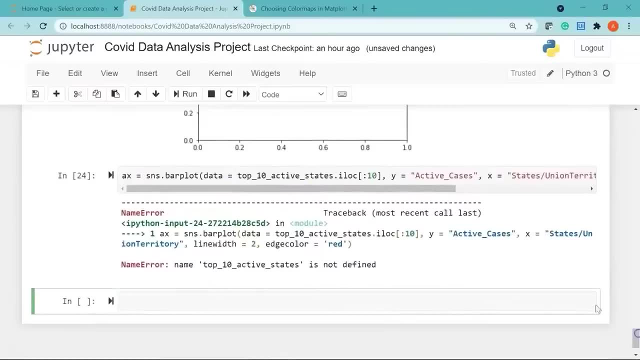 there's an error here. it says top 10 active states not found. let's go to the stop and see the exact. okay, so this is top 10 active cases. let me change it to cases here. now run it, okay. the x-axis also has a mistake. this should be state slash: union territory. 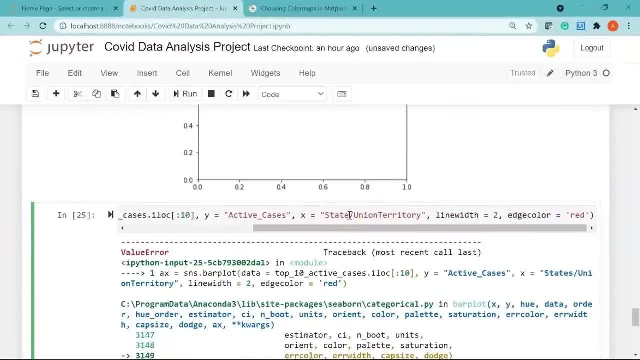 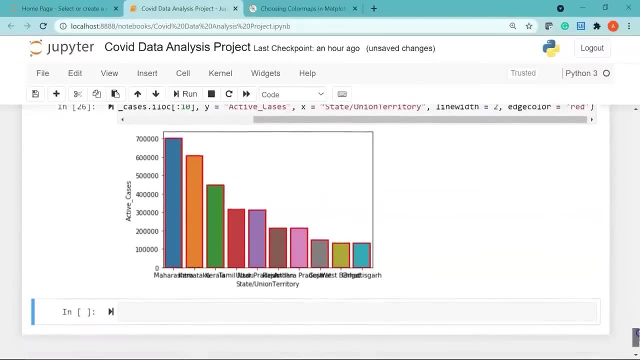 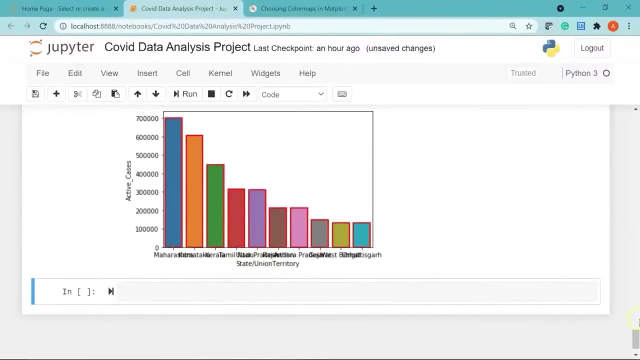 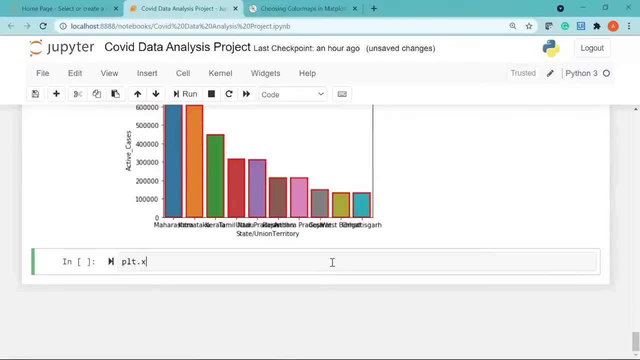 now let me run it. there you go. we have our plot created, but as you can see, here the labels of the different states and union territories are overlapping. so for that let me first pass in the x-axis here the x labels. i'll say plt, dot, x label and my x label would be states. then i'll say plt, dot, y label. 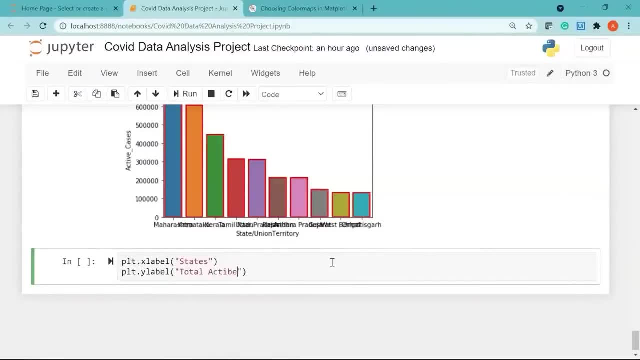 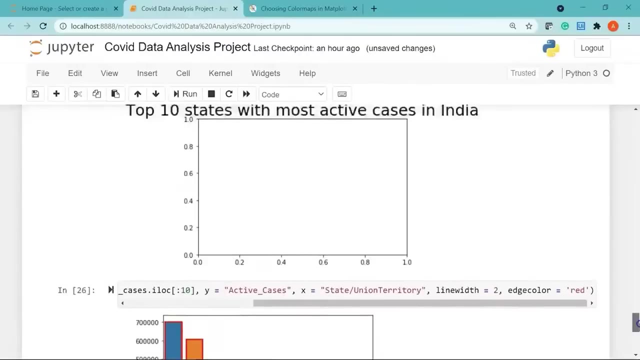 my y label will have the total active cases. and finally, i'll write plt dot show before i run it. let's say that i want to run it. let's run it before i run it. let's collate all the lines of code that we have written for our top 10 states. 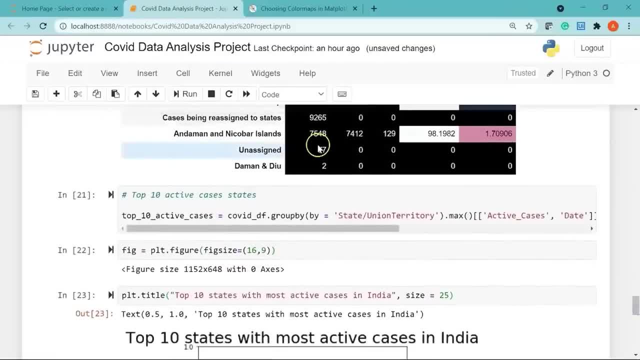 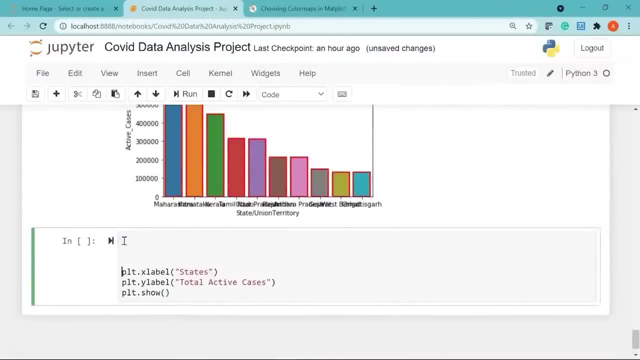 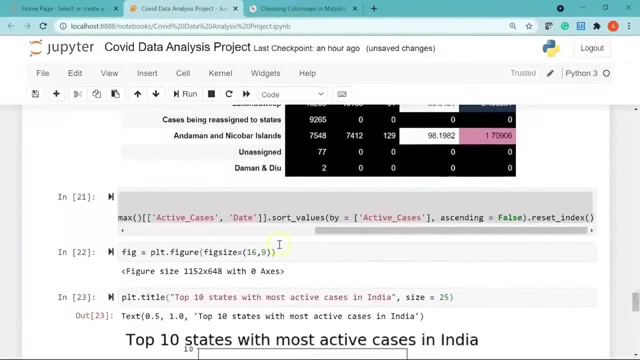 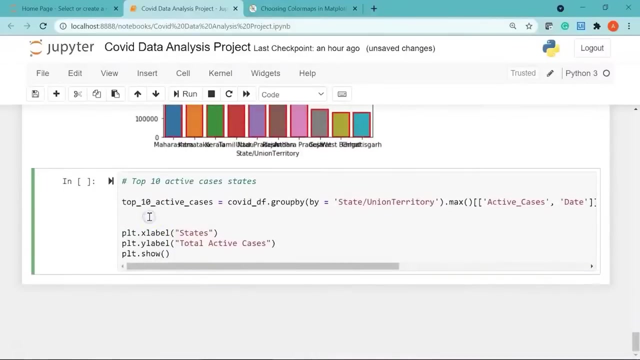 for most active cases in india- into one cell. so what i'll do is i'll just copy this and we'll keep adding in this cell itself. okay, i'll go to the top, next we'll copy my figure size and we'll paste it here. next let's take the title and put it here. 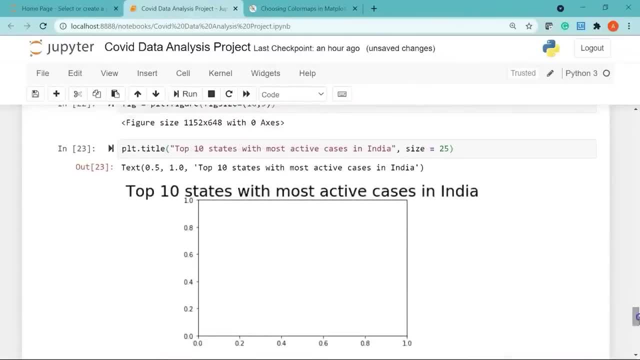 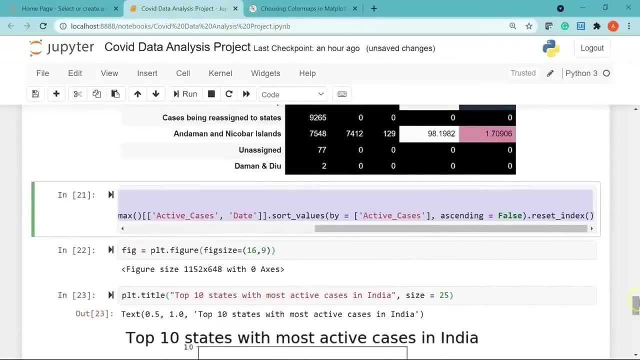 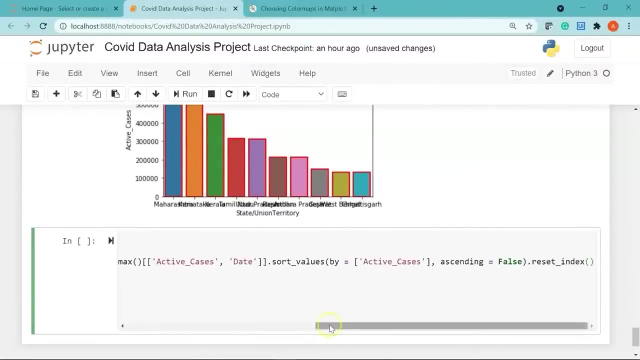 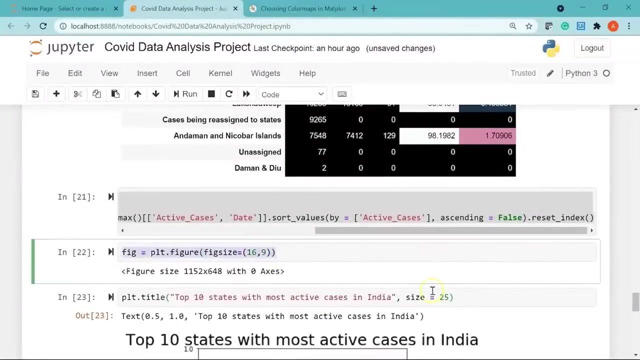 we have written for our top 10 states for most active cases in india into one cell. so what i will do is i will just copy this and will keep adding in this cell itself. ok, i will go to the top next, will copy my figure size and will 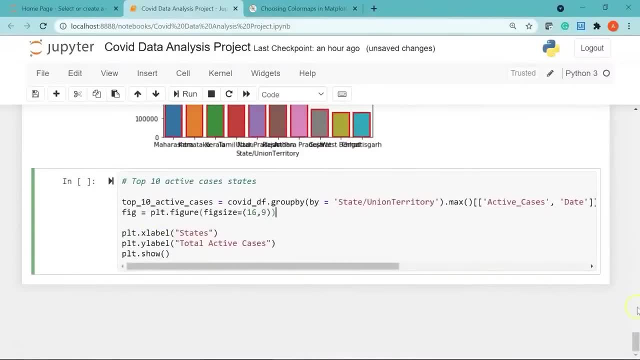 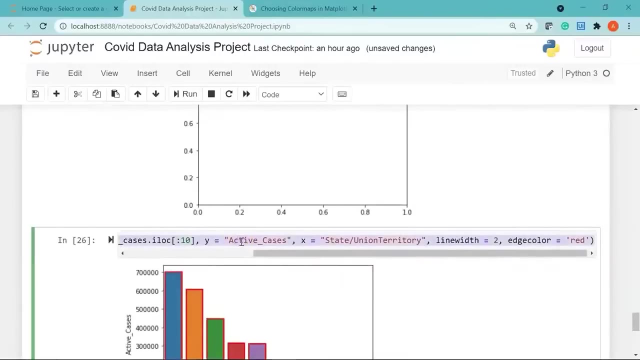 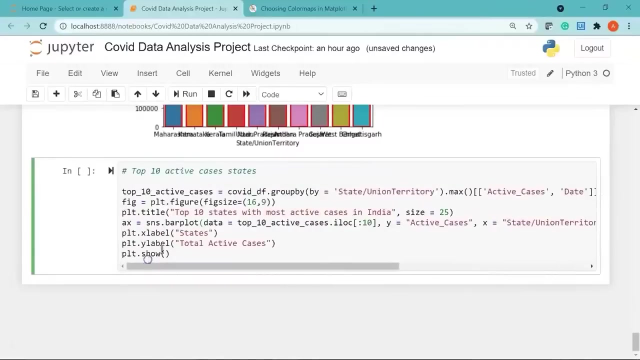 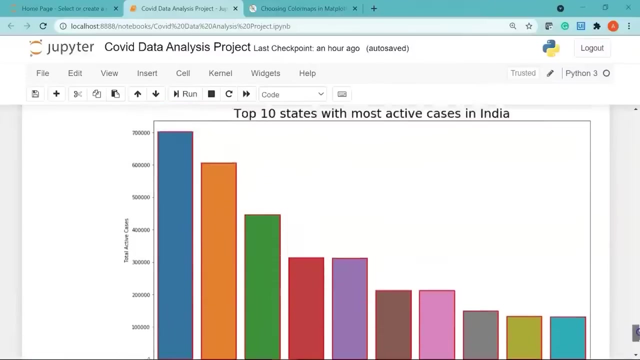 paste it here. next, lets take the title and put it here. give us piece and we are going to copy this cell and i will paste it here. alright, now its time to run it. there you go. you see it. here we have a nice bar plot ready on the. 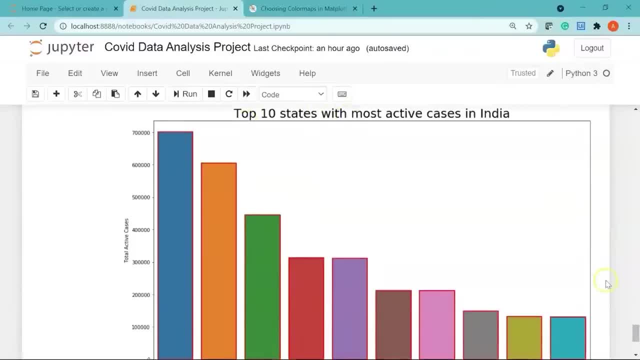 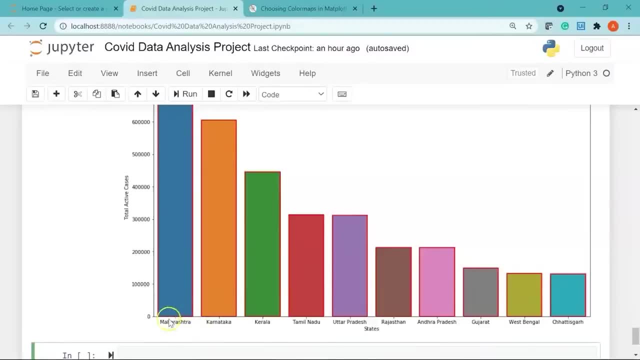 top you can see the title top 10 states with most active cases and you see the edges are in red colour. for all the bars on the x axis you have the different state names: maharashtra, karnataka, kerala. we also have andhra pradesh, gujarat, west bengal and chhattisgarh. 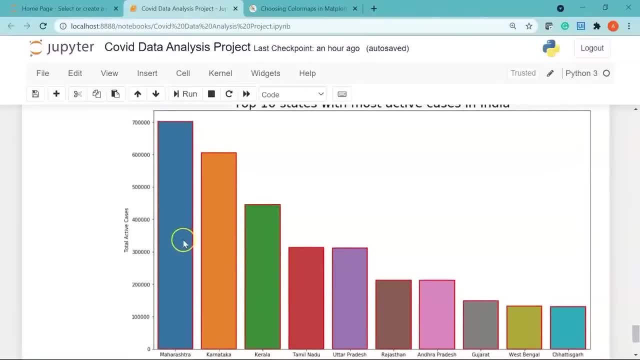 so, as you can see, maharashtra has the highest number of active cases based on our data, followed by karnataka, kerala and tamil nadu at second, third and fourth place respectively, and in the ninth place we have west bengal. in the tenth place we have 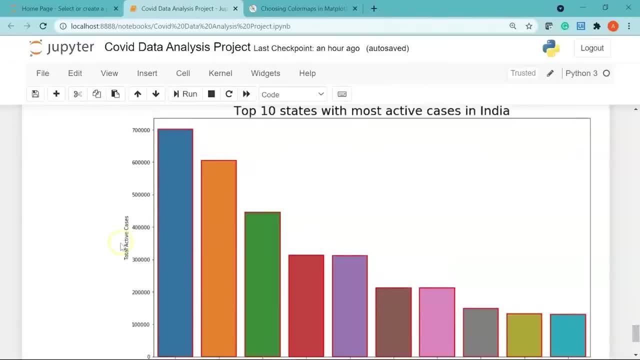 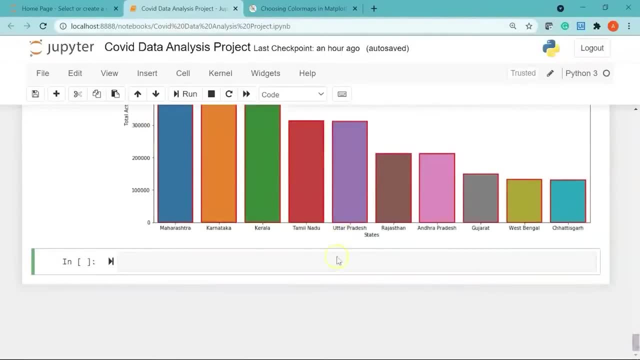 chhattisgarh, on the y axis, you can see the total active cases, which are in lakhs. ok, now moving ahead. now we will see the top 10 states based on the total number of deaths reported. so i will give a comment. top states with: 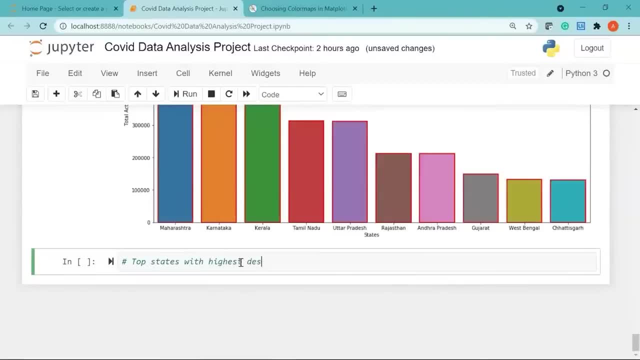 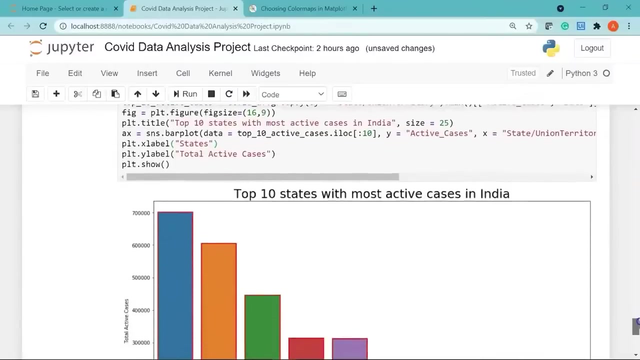 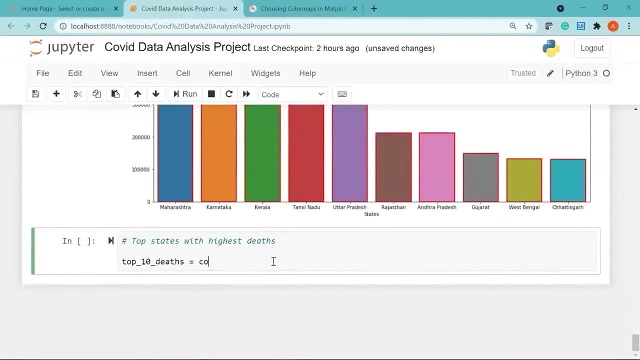 highest deaths. ok, so i will first create my variable saying top10 underscore deaths. this will be very similar to what we did here, just that we need to change a few column names. so instead of active cases, we will be using deaths. ok, so i will start with. 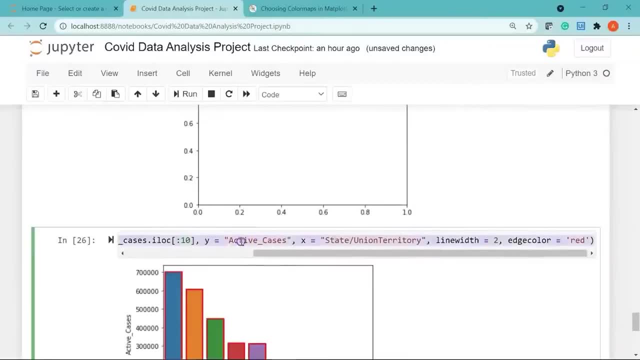 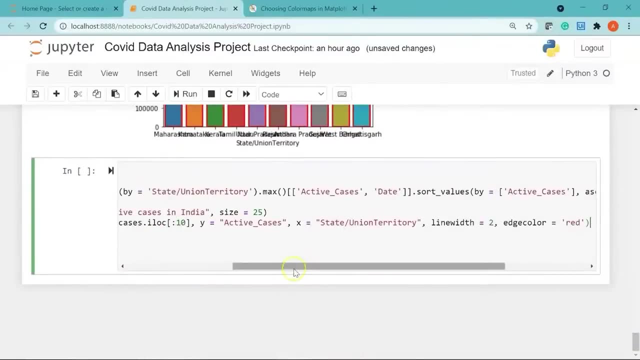 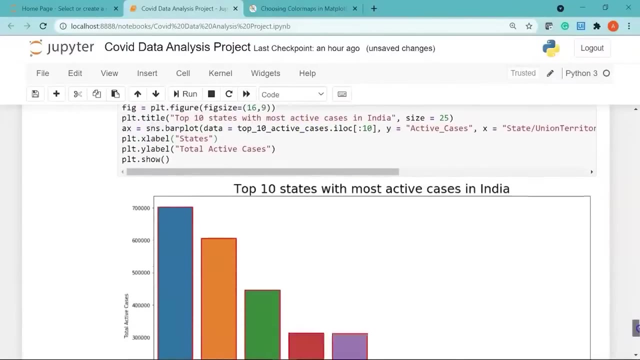 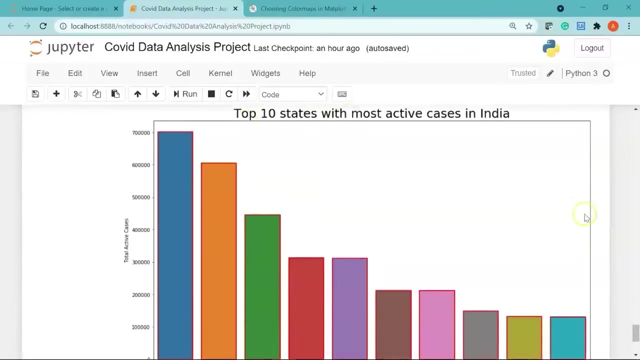 give us space and we are going to copy this cell and i'll paste it here. all right now it's time to run it. there you go. you see it here we have a nice bar plot ready. on the top you can see the title: top 10 states with most active cases. 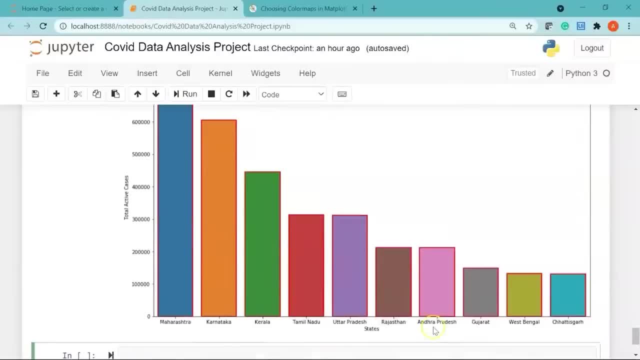 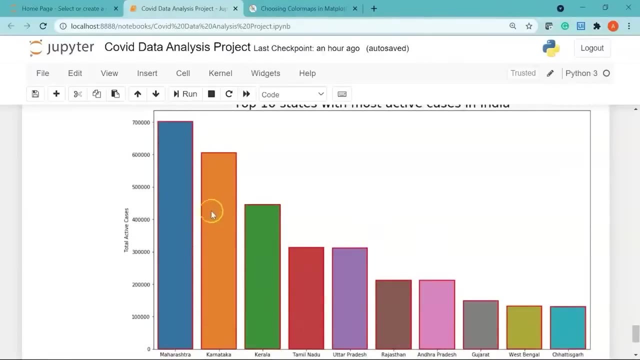 and you see the edges are in red color for all the bars. on the x-axis you have the different state names: maharashtra, karnataka, kerala. you also have andhra pradesh, gujarat, west bengal and chhattisgarh. so, as you can see, maharashtra has the highest number of active cases based on our data. followed by karnataka, kerala and tamilnadu at second, third and fourth place respectively, and in the ninth place we have west bengal. in the tenth place we have chhattisgarh. on the y-axis. you can see the total active cases. 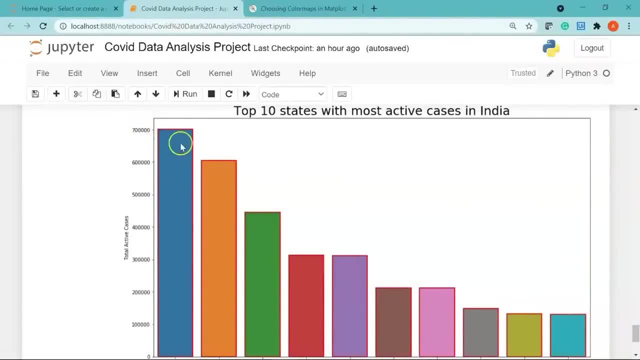 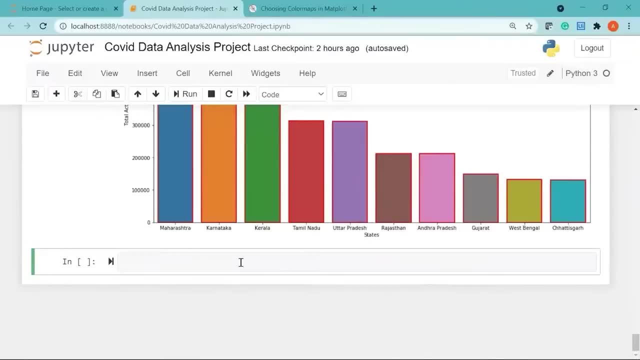 which are in lakhs. okay, now moving ahead. now we'll see the top 10 states based on the total number of deaths reported, so i'll give a comment: top states with highest deaths. okay, so i'll first create my variable saying top 10 underscore deaths. this will be very similar to 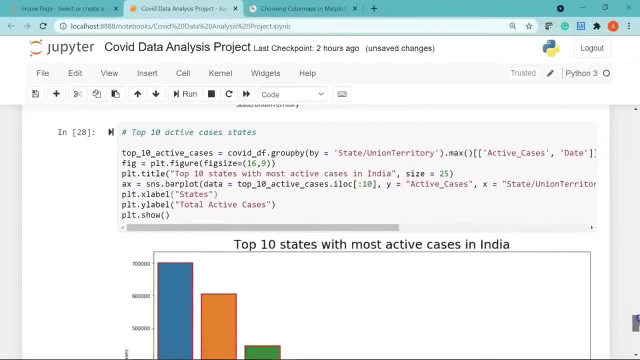 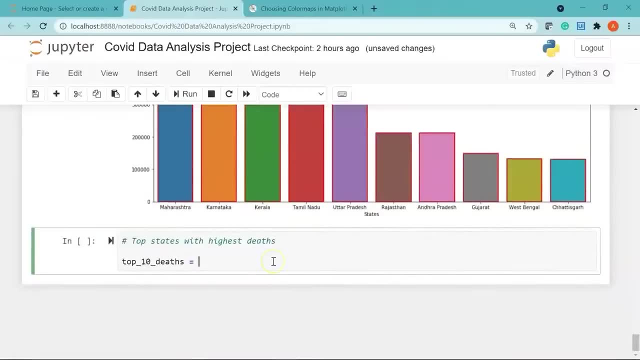 what we did here, just that we need to change a few column names. so instead of active cases, we'll be giving a function called deaths. okay, so i'll start with my data frame that is covered underscore df, followed by using the group by function, and i want to group my data based on the state slash. 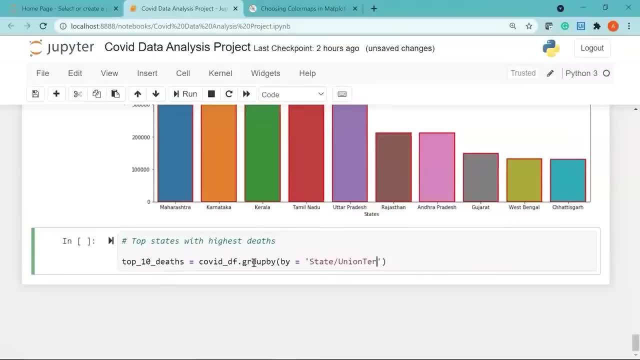 union territory column. then i'll choose the max function and within double square brackets I'll pass in my column names, deaths and date. let's make it consistent. I'll be using single quotes. okay, I'll say dot gonna short my result. therefore I'm using the short underscore values function I want. 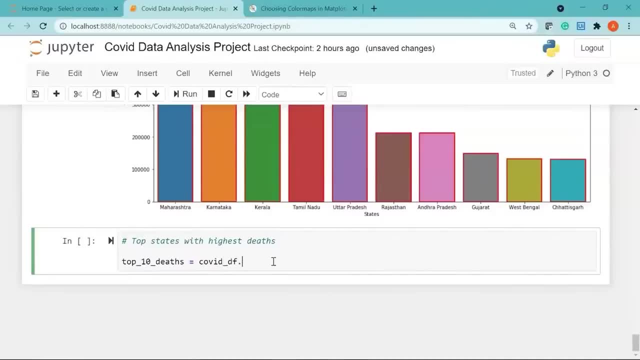 my data frame, that is, covid underscore df, followed by using the group by function. and i want to group my data based on the state slash union territory column. then i will choose the max function and within double square brackets i will pass in my column names, deaths and date. 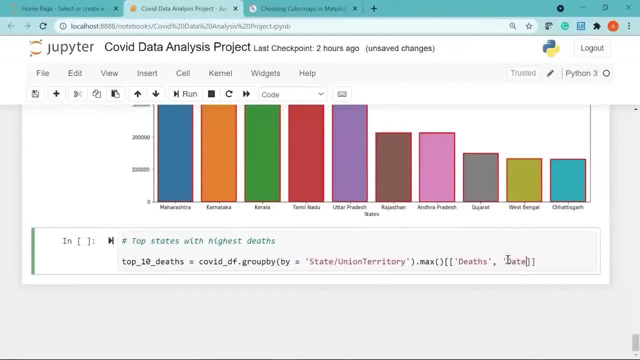 let's make it consistent. i will be using single quotes. ok, i will say dot, going to short my result. therefore, i am using the short underscore values function. i want to short it by deaths column. i will give another comma and say ascending equal to false, which means i want to. 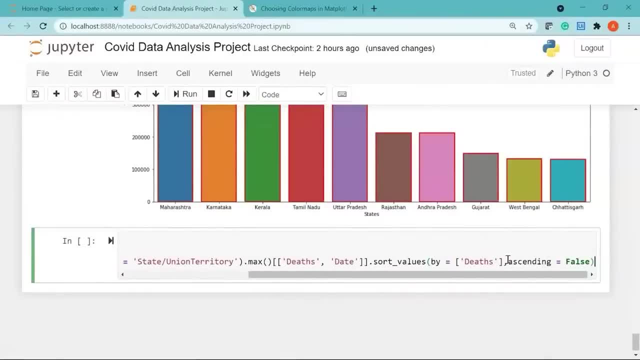 order, my result in descending order. then i will say dot reset underscore index. ok, after that i will give my figure size. i will say plt, dot figure and within brackets i will pass in my argument which is fig size equal to using a tuple. i will say 18 comma, let's say 5. 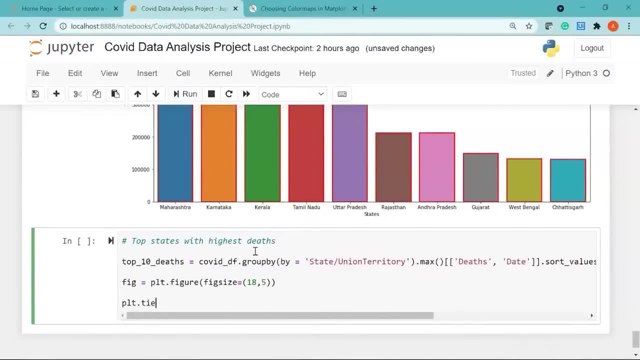 now let's give a title for that. i will use the title function which is present in the matplotlib library. i will say top 10 states with most deaths and let's give a size to the title 25. now it's time for us to give the axis labels. i will just scroll down. 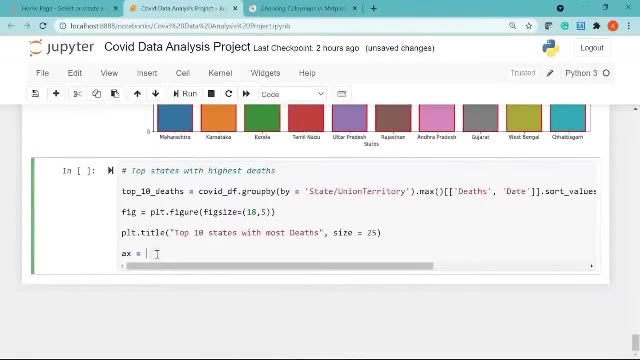 ok, so i will say ax equal to. again, this will be a barplot, so i am using my seaborn library, followed by the barplot function. my data will be top underscore 10 underscore deaths, which is this variable. i will give my index location, iloc. i am going to 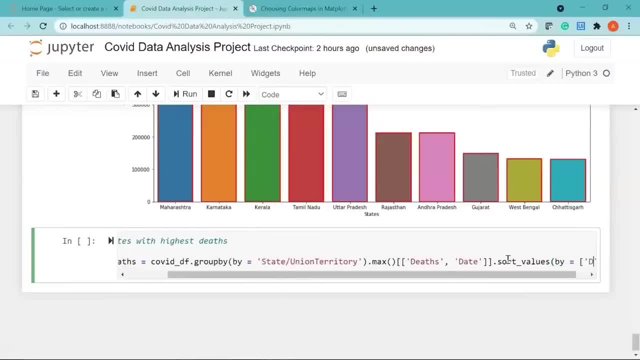 to short it by deaths column, I'll give another comma and say: ascending equal to false, which means I want to order my result in descending order. then I'll say dot reset underscore index. okay, after that I'll give my figure size as I'll say plt, dot figure, and within brackets I'll pass in my argument, which is fig size. 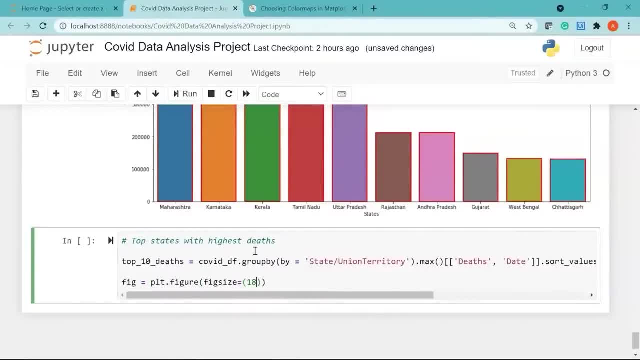 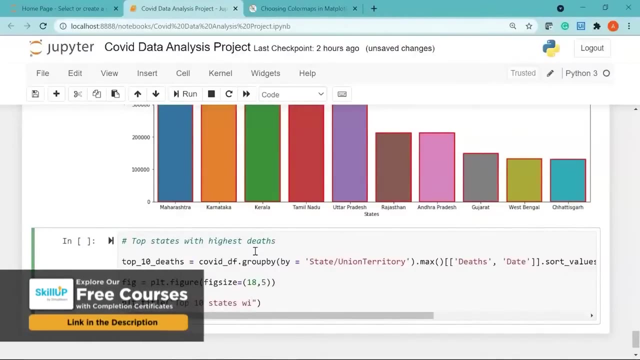 equal to using a tuple. I'll say 18 comma. let's say 5. now let's give a title for that. I'll use the title function which is present in the matplotlib library. I'll say top 10 states with most deaths, and let's give a size to the title 25. now it's time for us to give the axis. 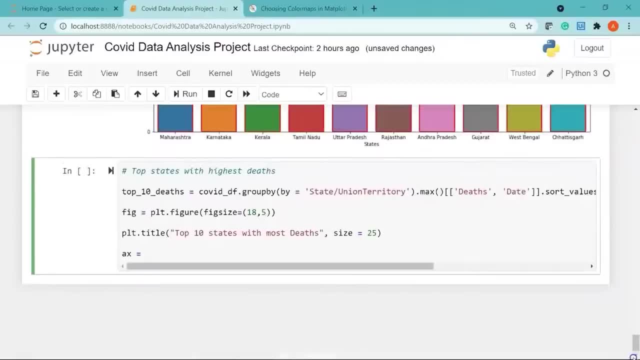 labels. I'll just scroll down. okay, so I'll say ax equal to. again, this will be a bar plot, so I'm using my seaborn library, followed by the bar plot function. my data will be top underscore 10 underscore deaths, which is this variable. I'll give my index location: i, ello c. I'm going to. 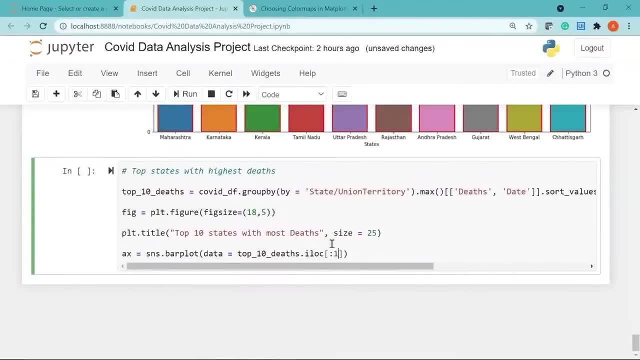 choose 12 states, the reason being there are some discrepancies in the data. I'll show you once I plot this result. so in the y-axis will have deaths column in the x-axis will take state slash Union territory. okay, give another comma and say line width equal to 2 and we'll. 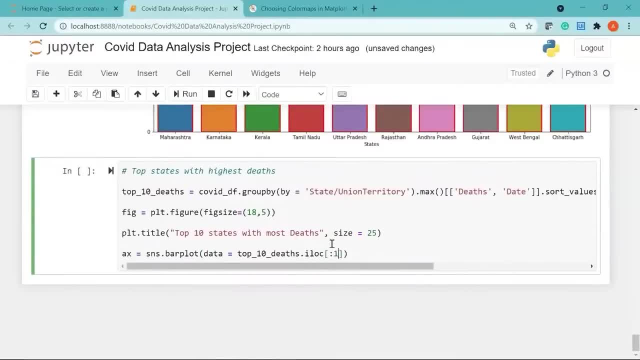 choose 12 states, the reason being there are some discrepancies in the data. i will show you once i plot this result. so in the y axis we will have deaths column. in the x axis we will take state slash union territory. ok, we will give another comma and say: 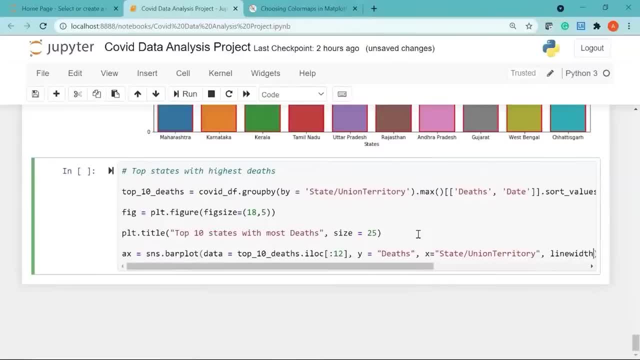 line width equal to 2 and we will give an edge column color to our bars, like we did here. so i will say edge color equal to, let's say, black. ok now, finally, we will give the x label, the y label, so i will say plt dot, x label. 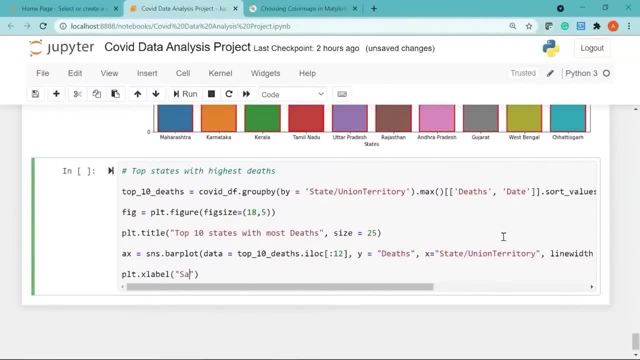 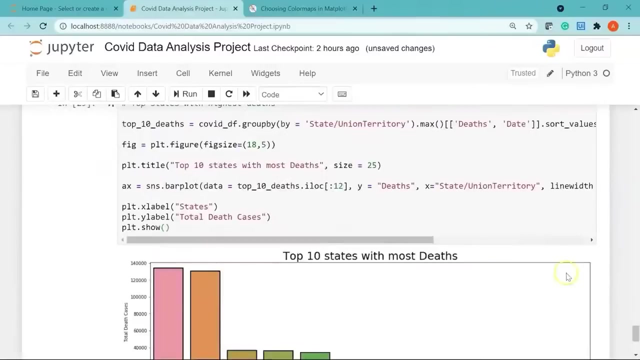 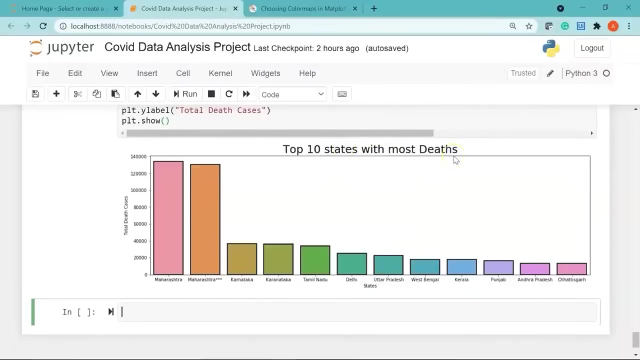 x label would be states. my y label will be total death cases. then i will write plt dot show. now let's run it. there you go. you can see here we have a nice bar plot. on the top we have the title: top 10 states with most deaths. 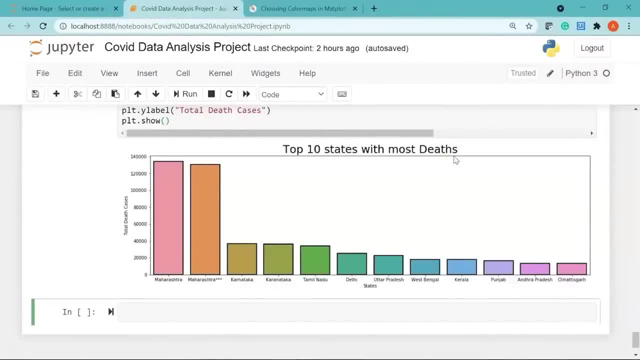 now, what i specifically wanted you to see was these discrepancies in the data. you can see here, maharashtra is repeated twice. even in our data that we collected from kegel, karnataka spelling has an error. you can see here. we have a few rows of information where karnataka is. 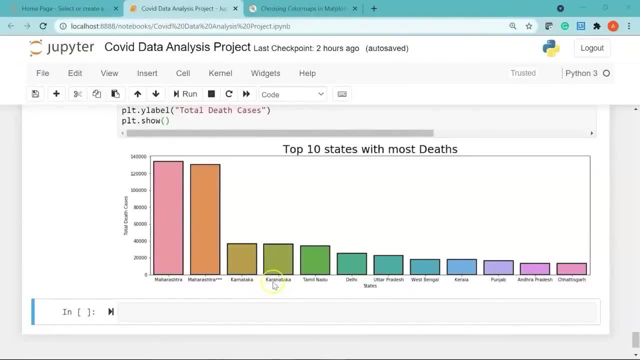 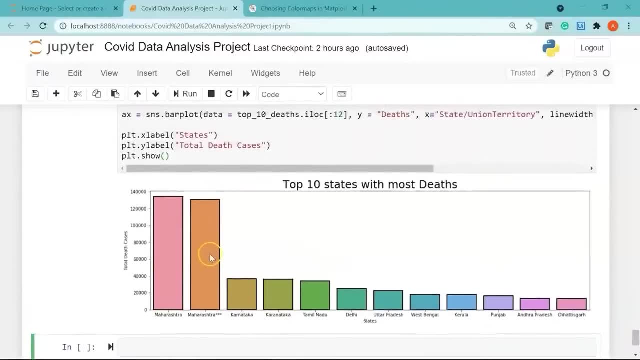 spelled as k-a-r-a-a-n. instead of k-a-r-n-a. alright, so to remove these two results or to ignore these two results. i had given my index location till 12, so we have maharashtra, karnataka, tamilnadu, delhi, then uttar pradesh, west bengal. 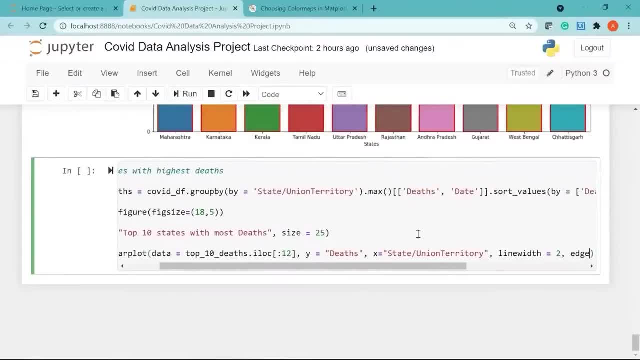 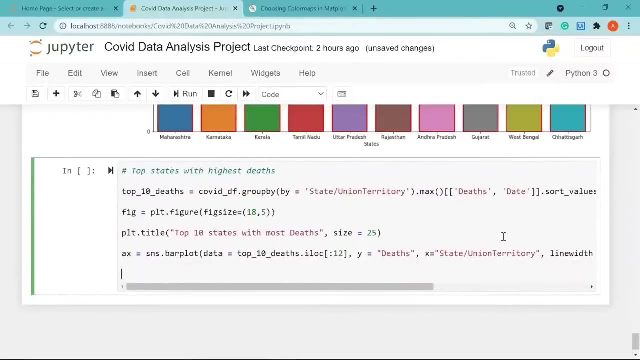 give an edge color to our bars, like we did here. so I'll say edge color equal to, let's say, black. okay, now finally, we'll give the X label the Y label. so I'll say PLT dot, X label. X label would be states, my Y label will be total death cases and I'll write PLT dot show. now let's run it. there you go. 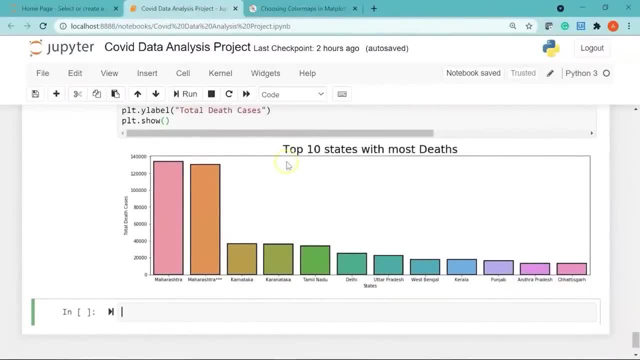 you can see, here we have a nice bar plot. on the top we have the title: top 10 states with most deaths. now, what I specifically wanted to do is: I wanted to show you how to do that. so I'm going to show you how to do that. so what I wanted you to see was these discrepancies in the data you can. 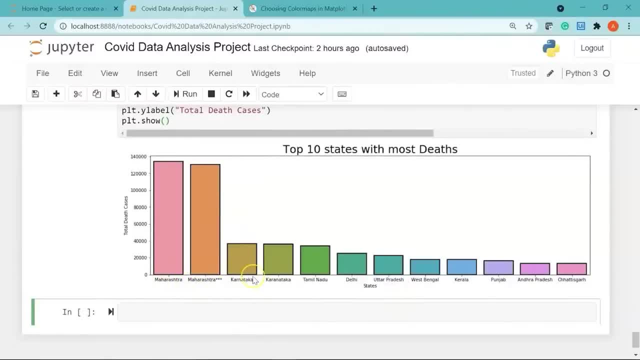 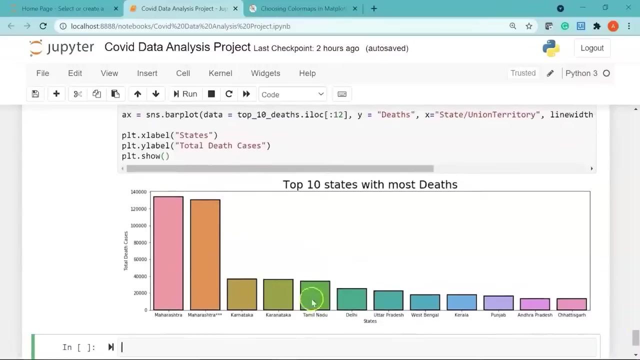 see here, Maharashtra is repeated twice. even in our data that we collected from Kegel, Karnataka spelling has an error. you can see here: we have a few rows of information where Karnataka is spelled as K-A-R-A-A-N instead of K-A-R-N-A. all right, so to remove these two results. 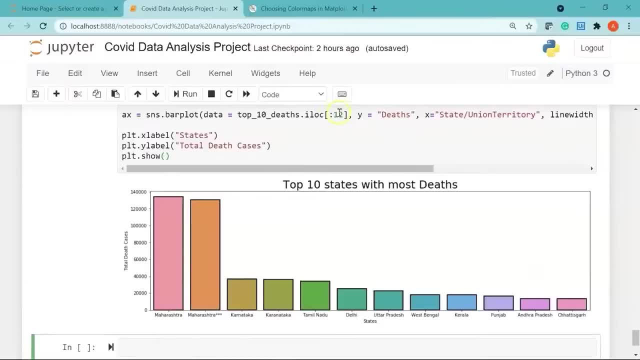 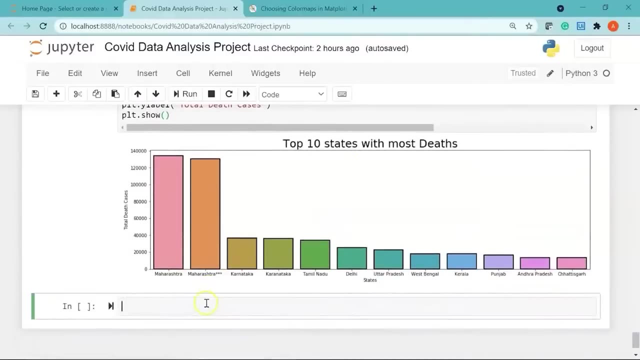 or to ignore these two results. I had given my index location till 12, so we have Maharashtra, Karnataka, Tamil Nadu, Delhi, then Uttar Pradesh, West Bengal, Kerala, Punjab, Andhra Pradesh and Chhattisgarh, with the states that have the most number of deaths reported. okay, 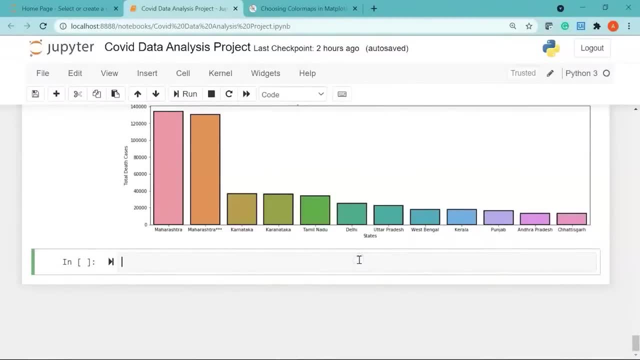 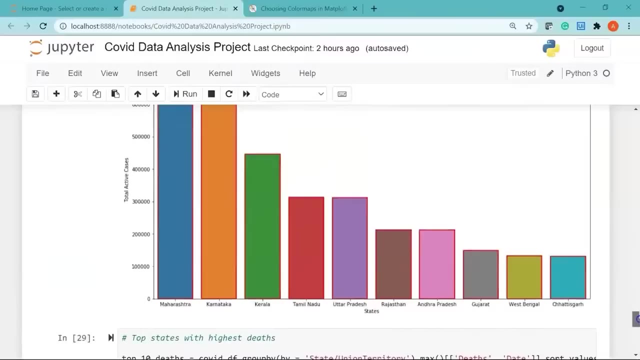 now we'll create a line plot to see the growth or the trend of active cases for top five states with most number of confirmed cases. so the states are maharashtra, karnataka, kerala, tamil nadu and utah pradesh. i can show you. so these are the states with highest number of active cases. 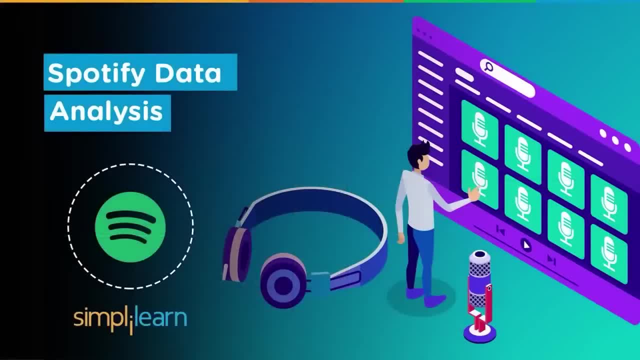 okay, hello everyone. welcome to today's video tutorial by simply learn. in this video, we are going to perform a really interesting data analysis using python on the spotify music streaming service platform data set. i'll also be asking you a few questions related to spotify during our discussion. please make sure to answer them in the comment section of the video. 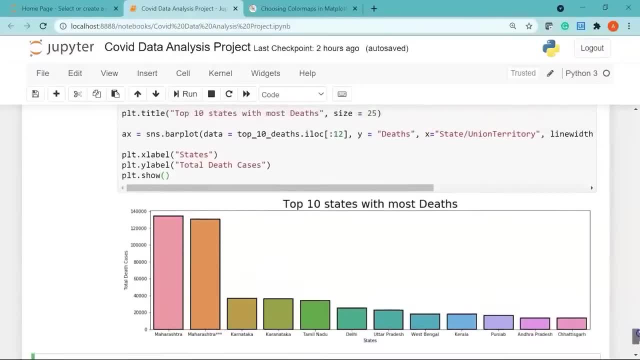 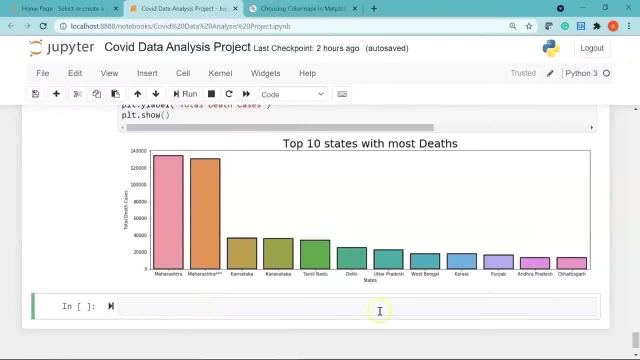 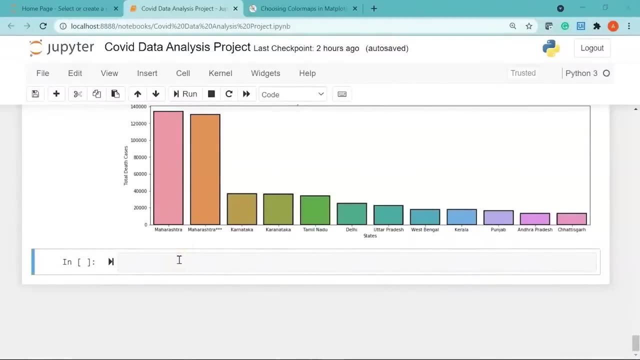 kerala, punjab, andhra pradesh and chhattisgarh, with the states that have the most number of deaths reported. ok, now we will create a line plot to see the growth or the trend of active cases for top 5 states with most number of confirmed cases. 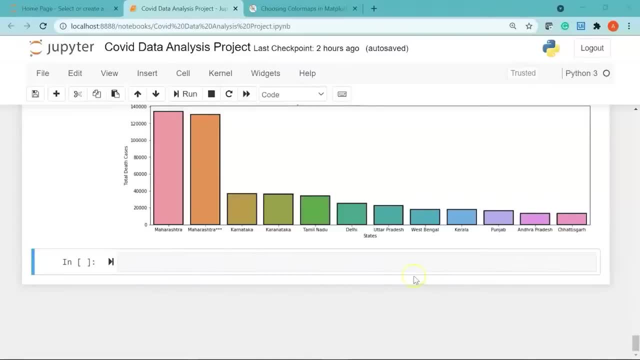 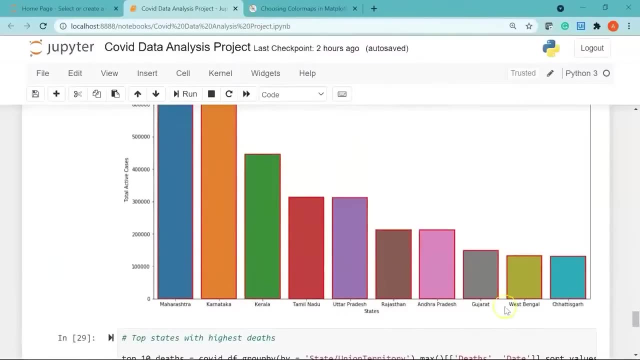 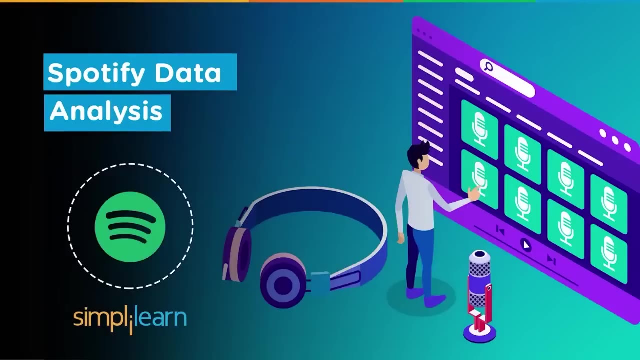 so the states are maharashtra, karnataka, kerala, tamilnadu and uttar pradesh. i can show you. so these are the states with highest number of active cases. ok, hello everyone. welcome to today's video tutorial. by simplylearn. in this video, we are going to perform a really interesting 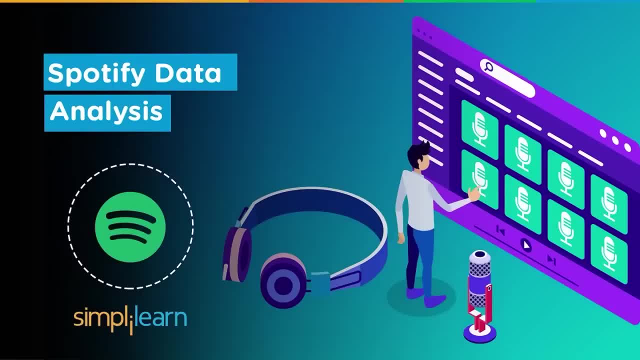 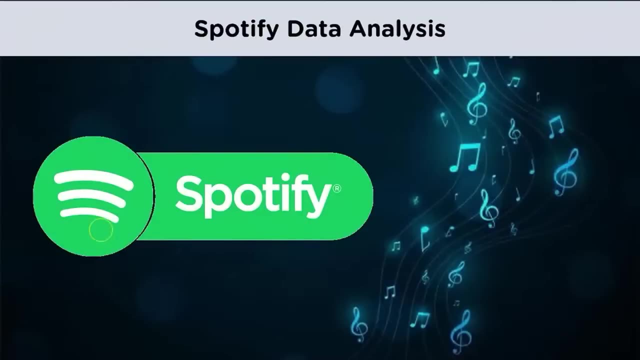 data analysis using python on the spotify music streaming service platform dataset. i will also be asking you a few questions related to spotify during our discussion. please make sure to answer them in the comment section of the video. so now let's get started. spotify is a swedish audio streaming and. 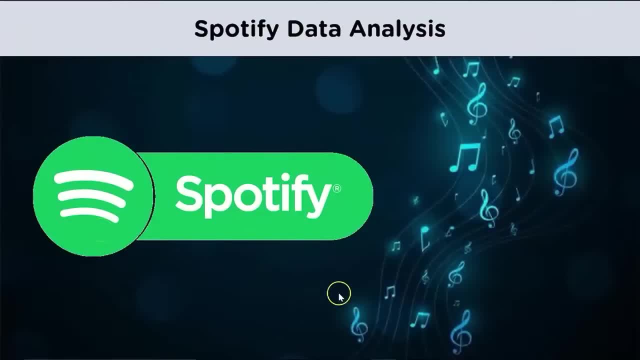 media services provider. founded in april 2006, it is the world's largest music streaming service provider and has over 381 million monthly active users, which also includes 172 million paid subscribers. the total number of downloads on the spotify app in the android store exceeded 1 billion. 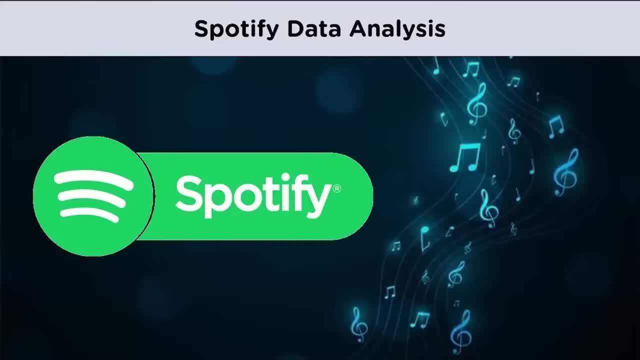 in may 2021. so millions of people listen to music all day. even i am hooked to music. as an analyst, what's better than exploring and quantifying data about music and drawing valuable insights? before i move ahead, i have a quiz question for you people. the name spotify. 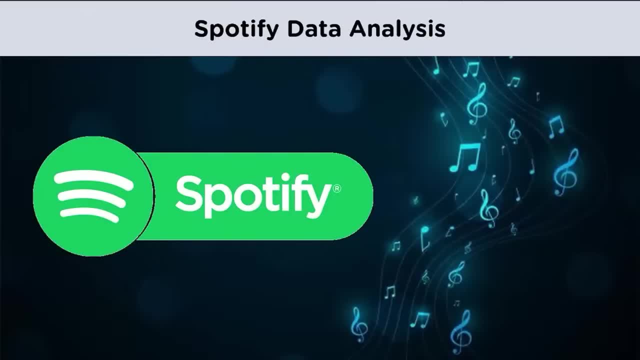 comes from a combination of two words, so which are those two words? please let us know your thoughts in the comment section below. i would like to repeat the question again. the name spotify comes from a combination of two words, so what are those two words? we would love to hear from you, so please put your. 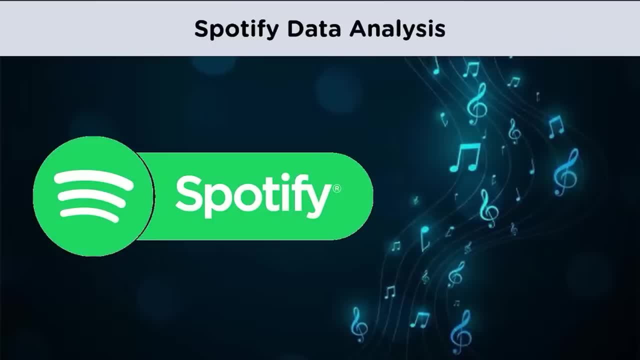 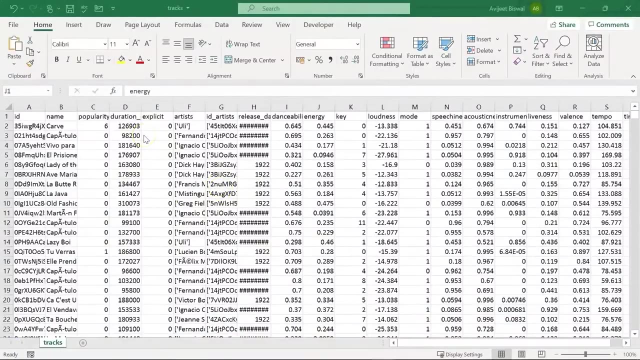 answers in the comment section below. now let's use python libraries and functions to analyze and visualize our dataset. first i'll show you the two datasets that we'll be using. so here is the first dataset that we'll be using for our demo, and then i have 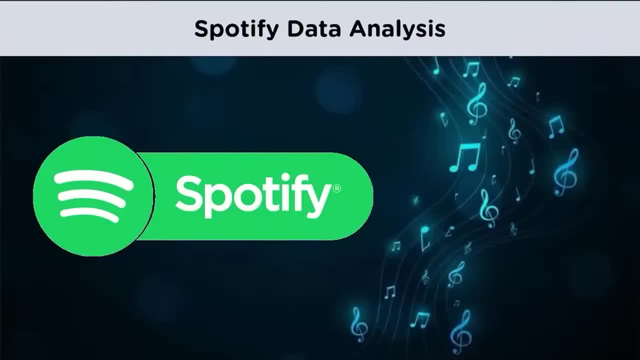 so now let's get started. spotify is a swedish audio streaming and media services provider founded in april 2006.. it is the world's largest music streaming service provider and has over 381 million monthly active users, which also includes 172 million paid subscribers. 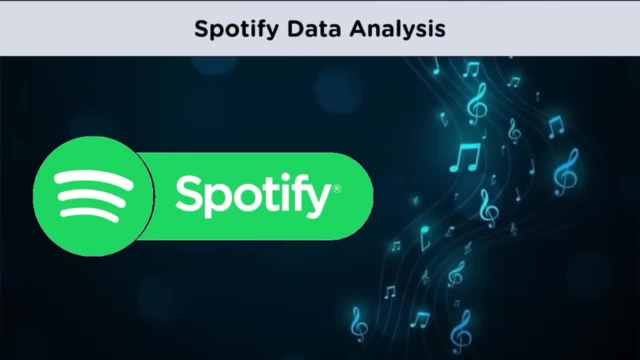 total number of downloads on the spotify app in the android store exceeded 1 billion in may 2021, so millions of people listen to music all day. even i am hooked to music. as an analyst, what's better than exploring and quantifying data about music and drawing valuable insights before i move ahead? 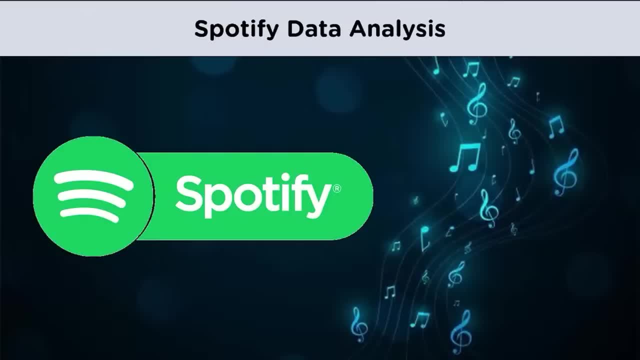 i have a quiz question for you people. the name spotify comes from a combination of two words, so which are those two words? please let us know your thoughts in the comment section below. i would like to repeat the question again: the name spotify comes from a combination of two. 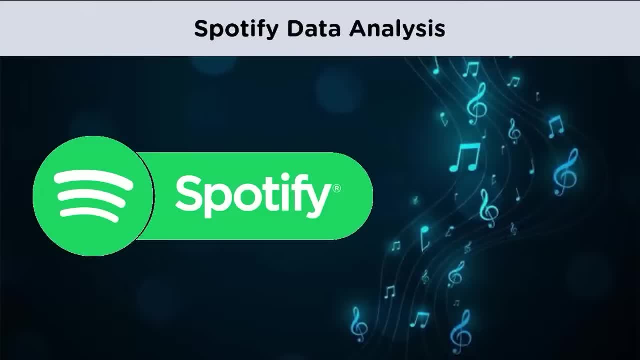 words. so what are those two words? we would love to hear from you. so please put your answers in the comment section below. now let's use python libraries and functions to analyze and visualize our data set. first, i'll show you the two data sets that we'll be using. 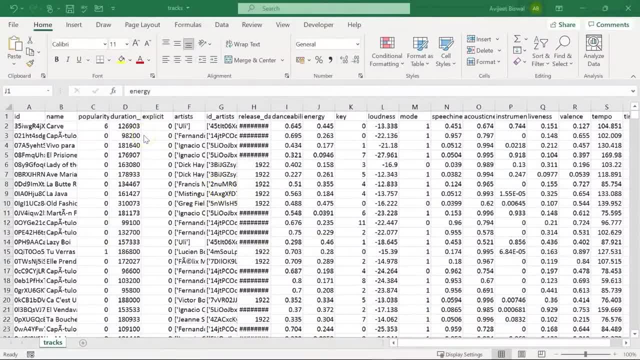 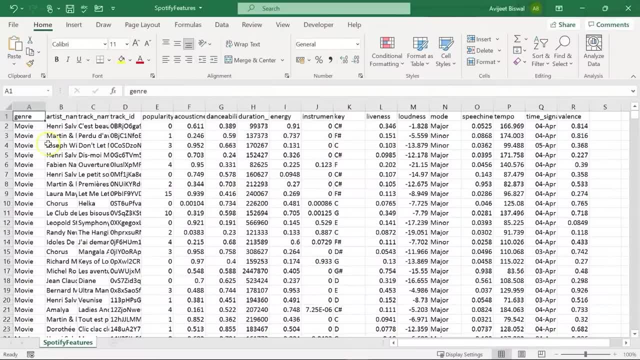 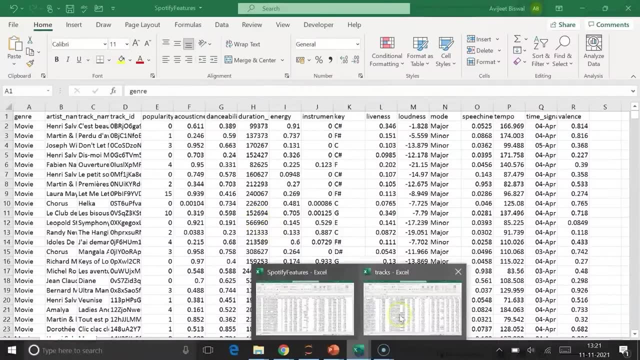 so here is the first data set that we'll be using for our demo, and then i have my second data set, called Spotify features, which is essentially about the genres of the different soundtracks. Now these data sets have been downloaded from kegelcom. Now the links to the data sets have been provided in the description box. please go ahead and. 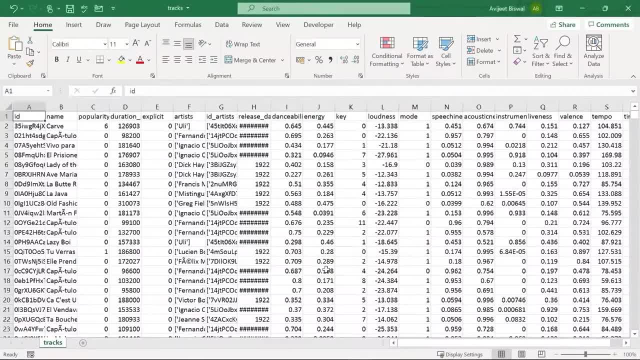 download them. Now. let me just go ahead and brief you about the columns that are present in our first data set, which is about tracks. We have our column A, which is ID. this is the unique ID for each of the songs. Then we have the name column, which is essentially the name of the song. 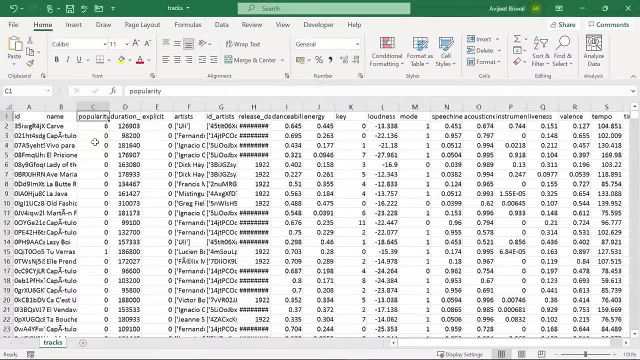 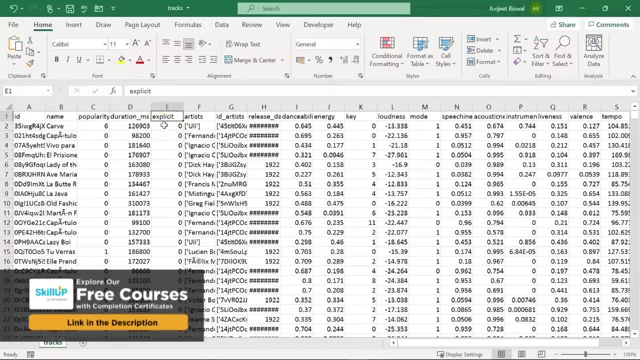 Then we have a column for popularity. so the popularity ranges from 0 to 100. Then we have duration in milliseconds. this is the duration of the track in milliseconds. Next we have a column called explicit. Now we are not bothered about this column because we are not going to use it in our 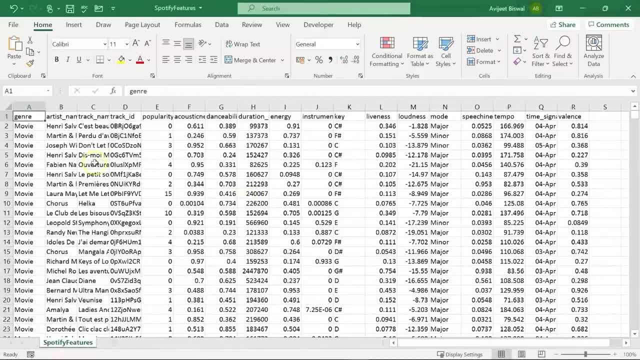 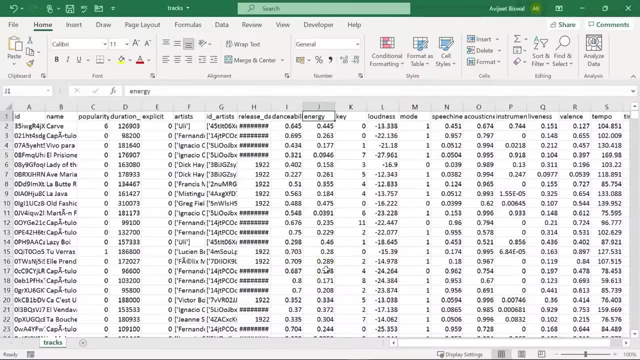 my second dataset called spotify features, which is essentially about the genres of the different soundtracks. now these datasets have been downloaded from kegelcom. now the links to the datasets have been provided in the description box. please go ahead and download them now. let me just go ahead and brief you. 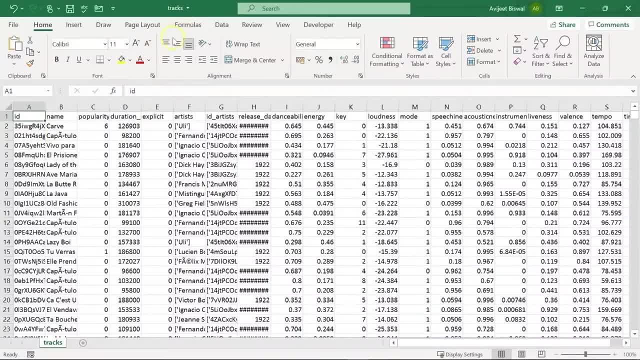 about the columns that are present in our first dataset, which is about tracks. we have our column a, which is id- this is the unique id for each of the songs. then we have the name column, which is essentially the name of the song. then we have a column for: 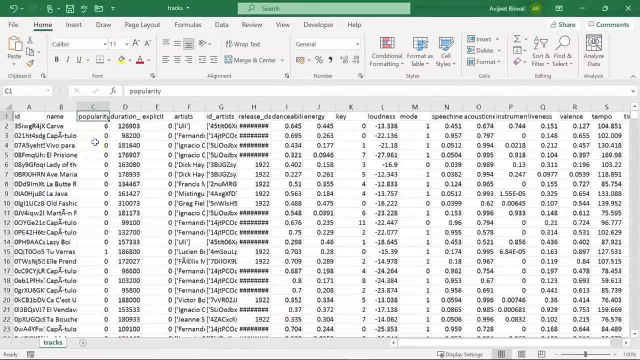 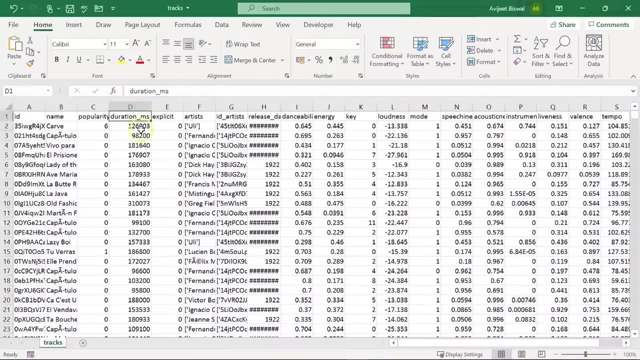 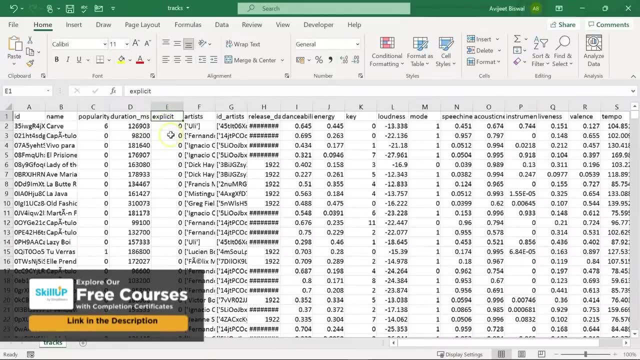 popularity. so the popularity ranges from 0 to 100. then we have duration in milliseconds. this is the duration of the track in milliseconds. next we have a column called explicit. now we are not bothered about this column because we are not going to use it in our 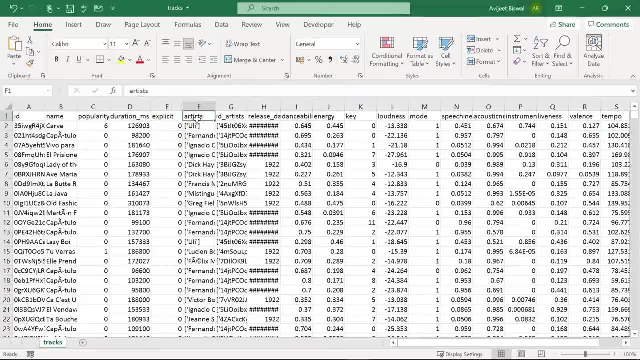 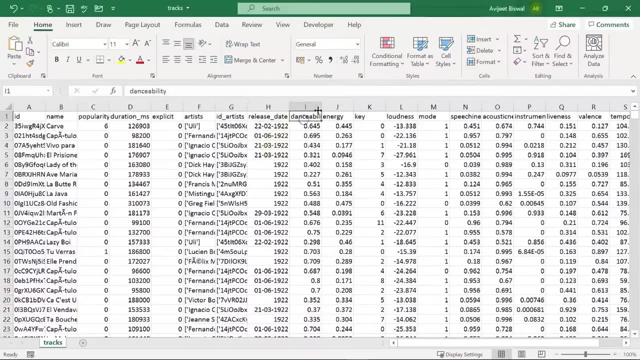 analysis. then we have artist, so the name of the artist who has composed or sung the song. then we have id of the artist, then we have a column for release date, which is basically the date on which the song was released. then we have a column for danceability. 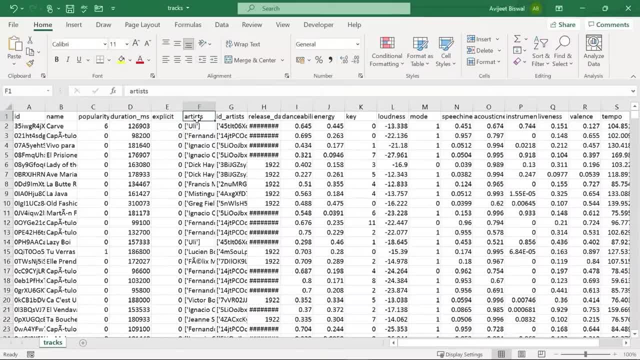 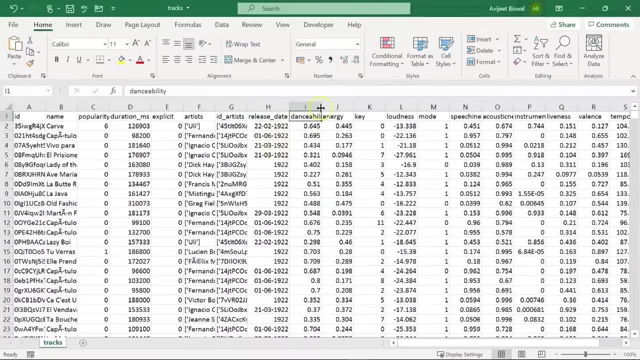 analysis. then we have artist, so the name of the artist who has composed or sung the song. then we have id of the artist, then we have a column for release date, which is basically the date on which the song was released. then we have a column for danceability. so this describes how suitable. 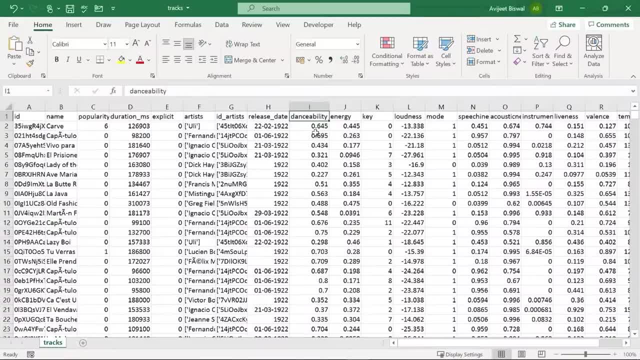 a track is for dancing, based on a combination of musical elements such as tempo, rhythm, stability, beat strength and overall regularity. the value ranges between 0 and 1. next we have a column for energy, so the energy is a measure between 0.0 to 1.0 and represents a perceptual measure of. 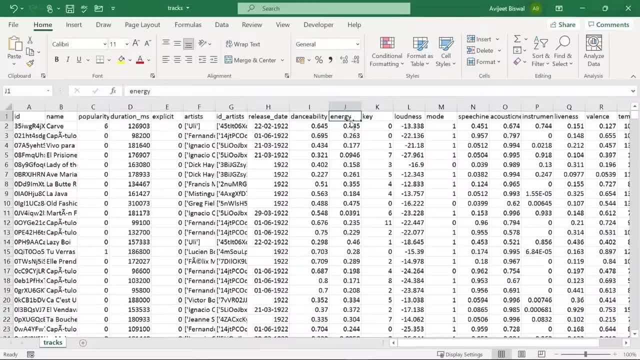 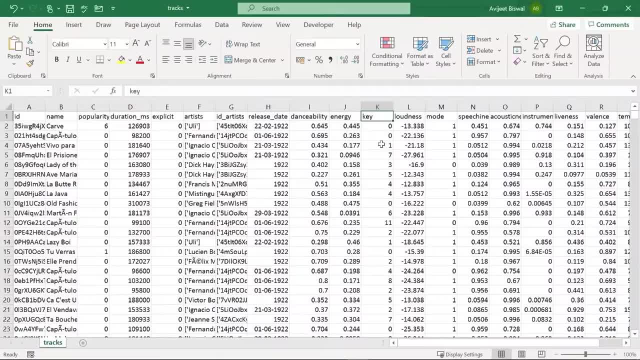 scale of song. that forms the basis of a song. there are 12 keys ranging from 0 to 11.. moving ahead we have loudness, so the overall loudness of the track in decibels it ranges from minus 60 to 0 decibels. then we have mode, so songs can be classified as major and minor. 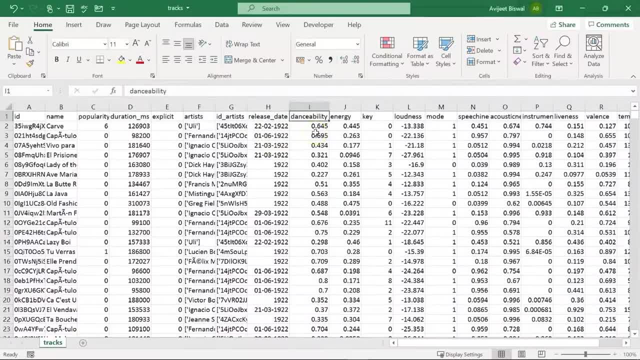 so this describes how suitable a track is for dancing, based on a combination of musical elements such as tempo, rhythm, stability, beat strength and overall regularity. the value ranges between 0 and 1. next we have a column for energy, so the energy is a measure between: 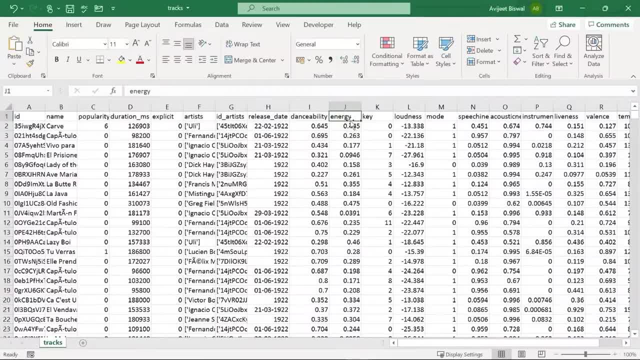 0.0 to 1.0 and represents a perceptual measure of intensity and activity. typically the energetic tracks feel fast, loud and noisy. higher the value, the more energetic is the song. then we have a column for key. so key is the pitch notes or scale of. 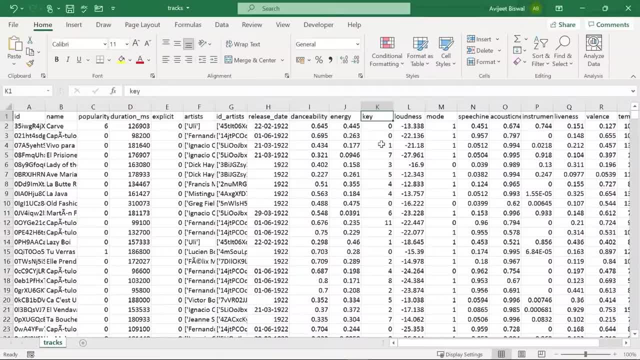 song that forms the basis of a song. there are 12 keys, ranging from 0 to 11. moving ahead. we have loudness, so the overall loudness of the track in decibels it ranges from minus 60 to 0 decibels. then we have mode. 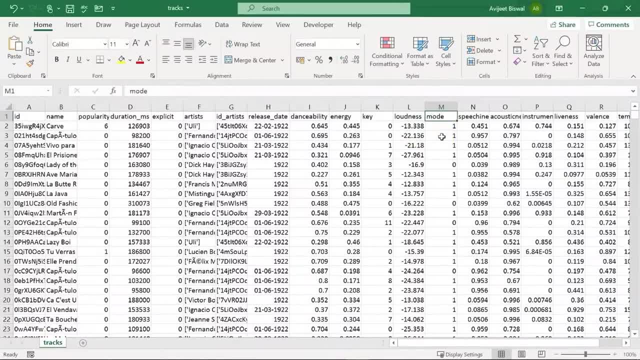 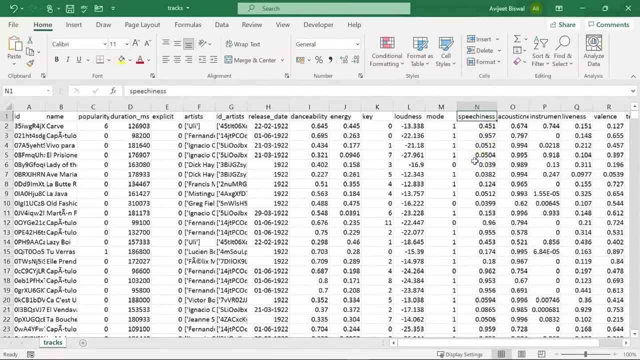 so songs can be classified as major and minor: 1.0 represents major or 1 represents major and 0 represents minor. next we have speechiness. so speechiness recognizes the presence of spoken words in a track. more exclusive speech, like the recording example, show, audiobook or poetry, the 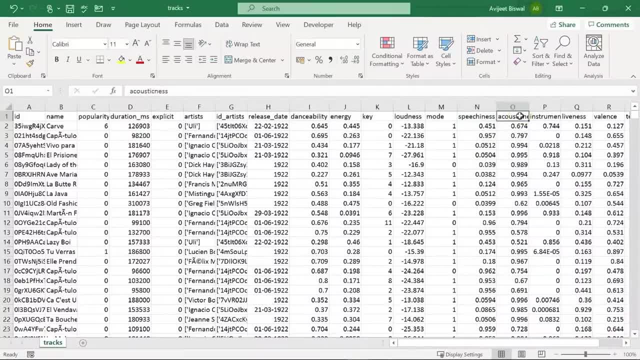 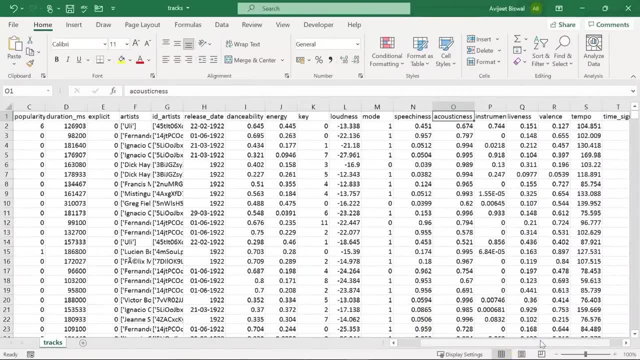 closer to 1.0 the attribute value. then we have a column for acousticness, so a confidence measure of 0 to 1 of whether the track is acoustic or not. so 1.0 represents high confidence. the track is acoustic, then we have other information about. 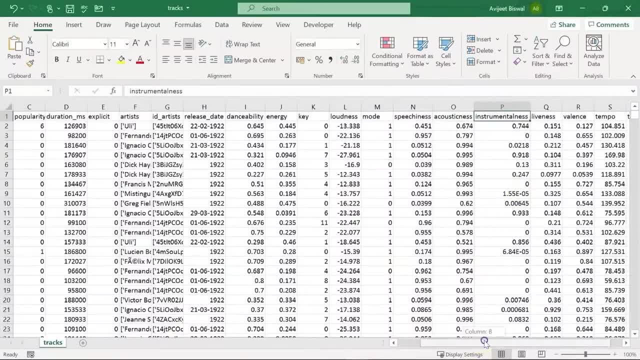 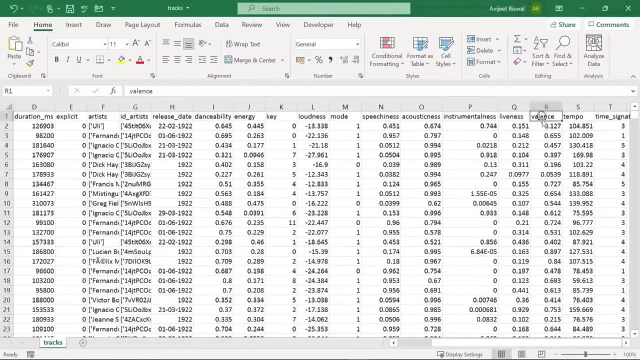 instrumentalness. then we also have a column for liveness, so liveness detects the presence of an audience in the recording. then we have a column for valence, so valence is a measure between 0.0 to 1.0 and describes the musical. 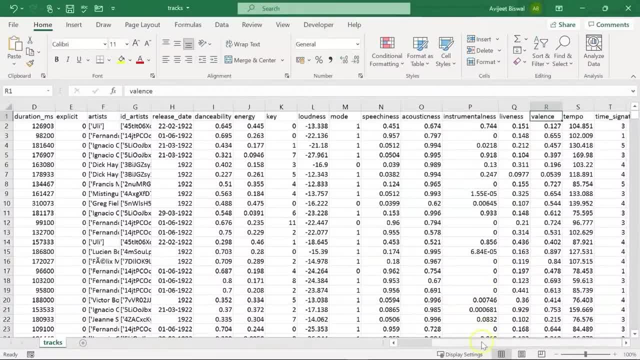 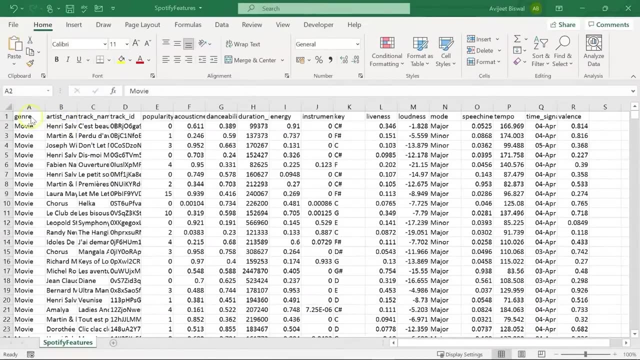 positiveness conveyed by a track or a song. and finally, we have the columns for tempo and time signature. now, even in the second dataset, we have almost the same columns, just that we have an additional column that is about the genre of the songs present in the dataset. cool, 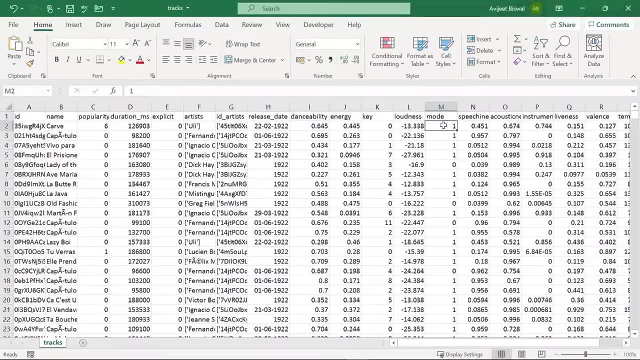 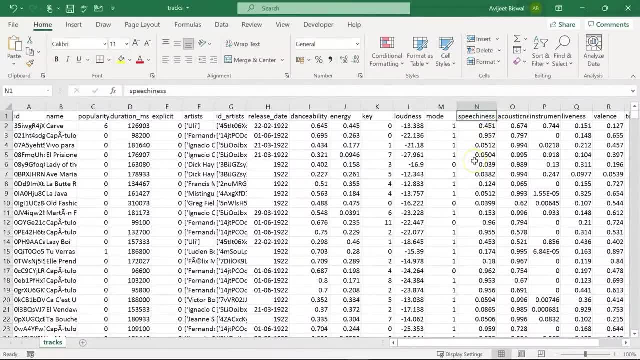 1.0 represents major, or 1 represents major and 0 represents minor. so those are what we are looking at in this video. so a该 lets jump into talking about each part of the track. next we have Speechiness. so speechiness recognizes the presence of spoken words in a track. 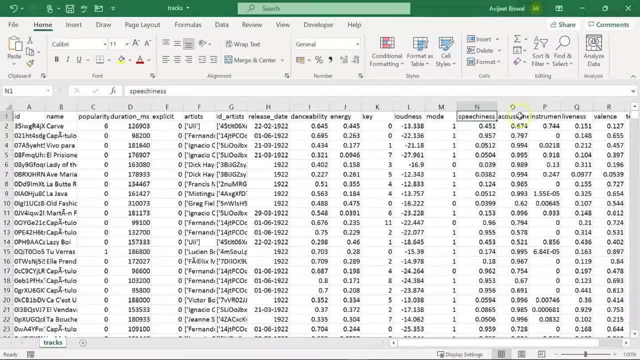 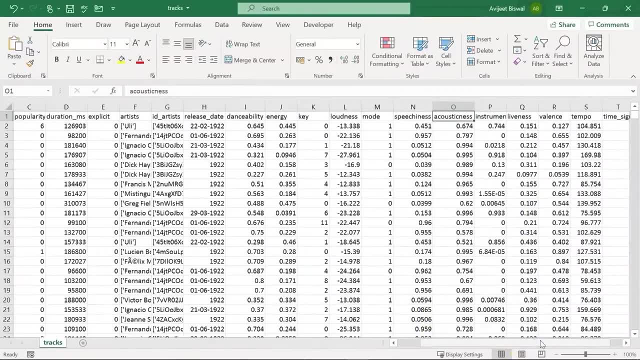 more exclusive speech, like the recording example: talk show, audiobook or poetry. they are closer to 1.0, the attribute value. then we have a column for acoustic notes, acoustic or not, so 1.0 represents high confidence. the track is acoustic, then we have other. 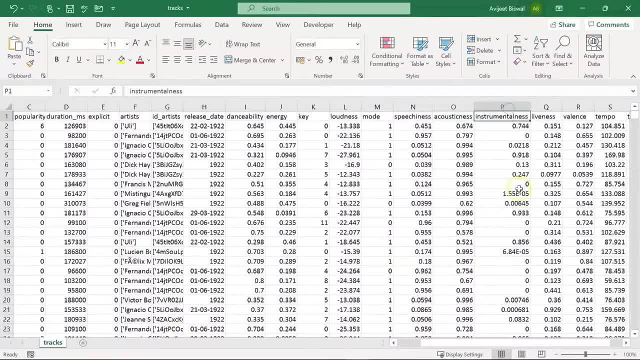 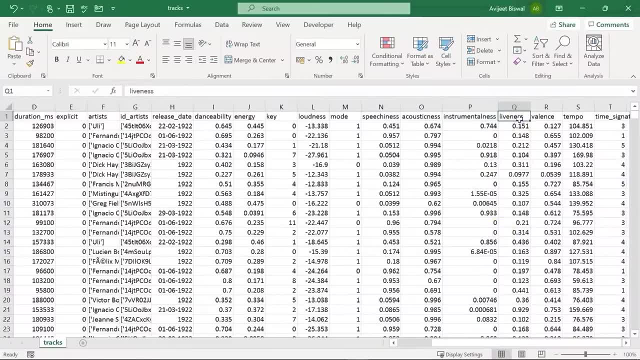 information about instrumentalness. then we also have a column for liveness, so liveness detects the presence of an audience in the recording. then we have a column for valence, so valence is a measure between 0.0 to 1.0 and describes the musical positiveness conveyed by a track or a. 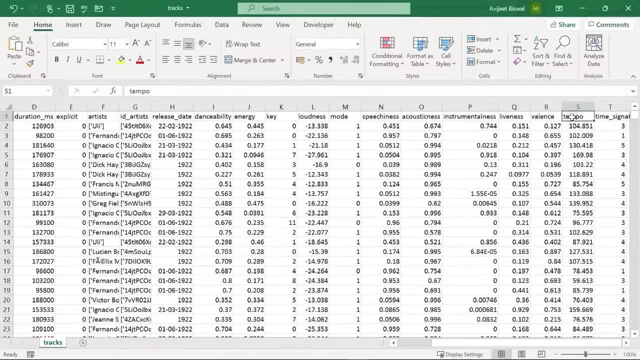 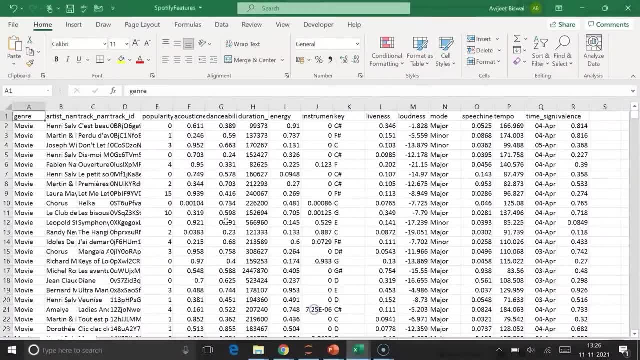 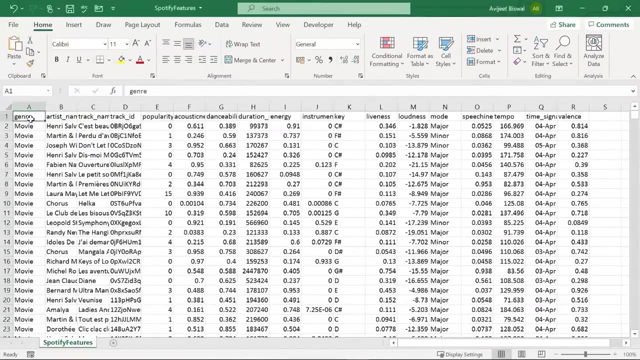 song. and finally, we have the columns for tempo and time signature. now, even in the second data set, we have almost the same columns, just that we have an additional column that is about the genre of the songs present in the data set. cool, now let's head over to our jupyter notebook and 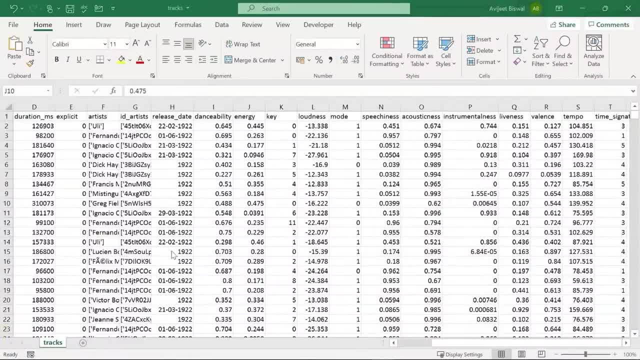 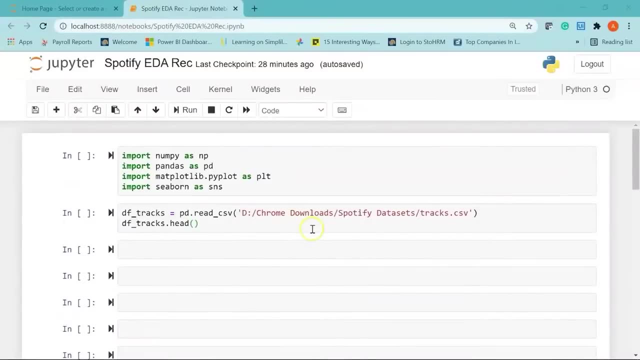 we'll start with our analysis. okay, so one more thing to remember: our data data has information from 1922 onwards, so all the songs from 1922 till 2021, cool, okay. so i am on my jupyter notebook so you can see i have a few cells that have already been filled up. so we'll start with. 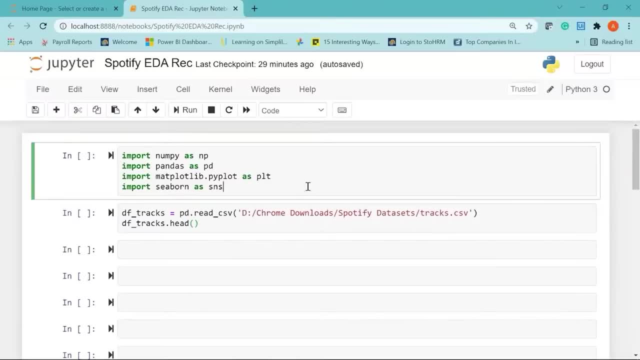 our analysis. first of all, let's go ahead and import the necessary libraries. so i'm importing numpy, pandas, matplotlib and seaborn for my analysis and then we'll start with our analysis and visualization. i'll hit shift, enter to import the libraries, all right, and in the next cell i'm 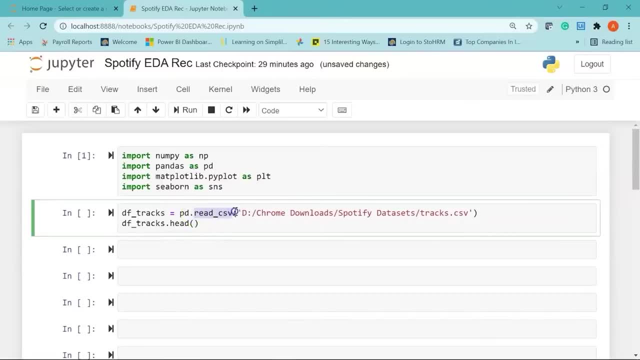 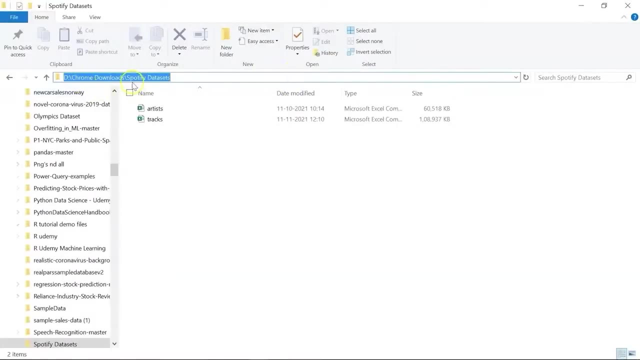 going to load my data set using the pandas read underscore csv function. i have my location already put here. let me show you the location where the data files or the data sets are located. so this is my location. under chrome downloads, i have a folder called spotify datasets. 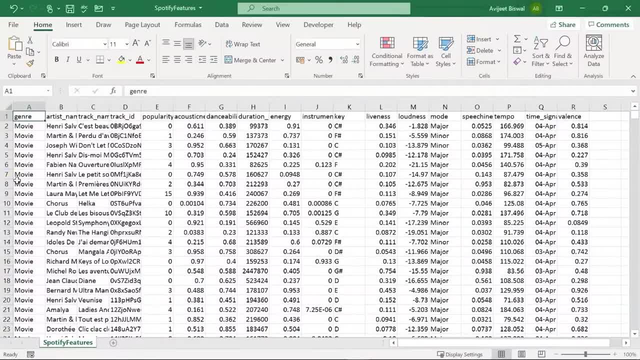 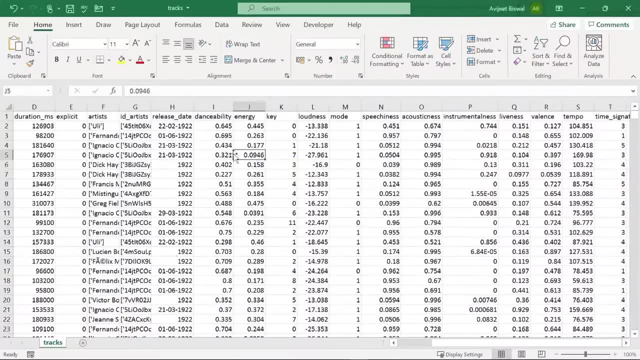 now let's head over to our jupiter notebook and we'll start with our analysis. ok, so one more thing to remember. our data has information from 1922 onwards, so all the songs from 1922 till 2021. cool, ok, so i am on my jupiter notebook. 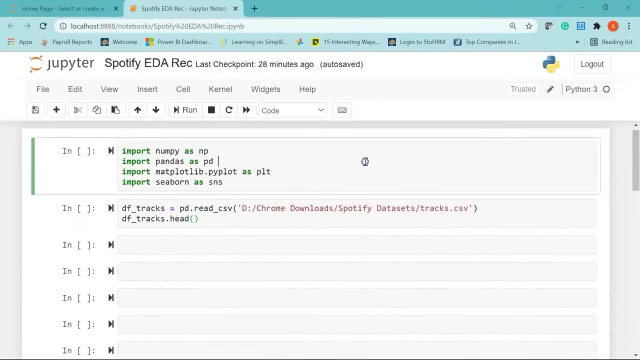 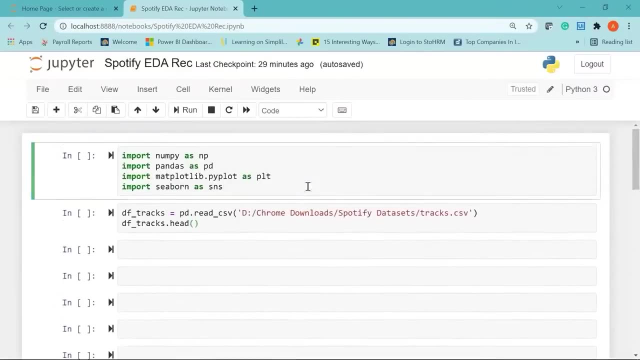 so you can see i have a few cells that have already been filled up, so we'll start with our analysis. first of all, let's go ahead and import the necessary libraries. so i am importing numpy, pandas, matplotlib and seaborn for my analysis and visualization. i'll hit. 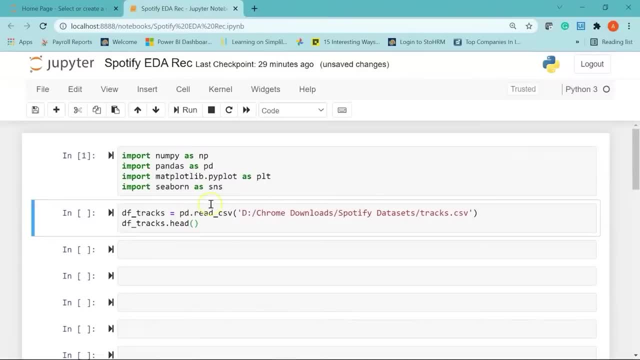 shift, enter to import the libraries. alright, and in the next cell i am going to load my dataset using the pandas read underscore csv function. i have my location already put here. let me show you the location where the data files or the datasets are located. so this is my location under chrome downloads. 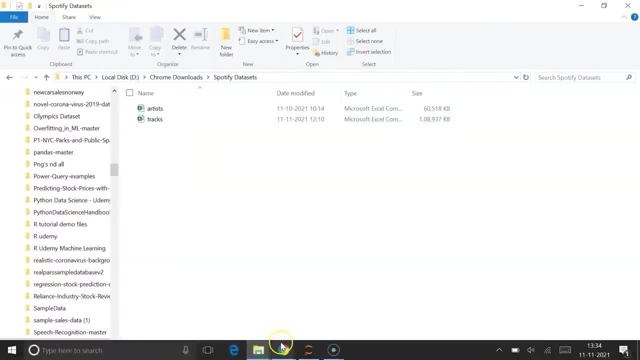 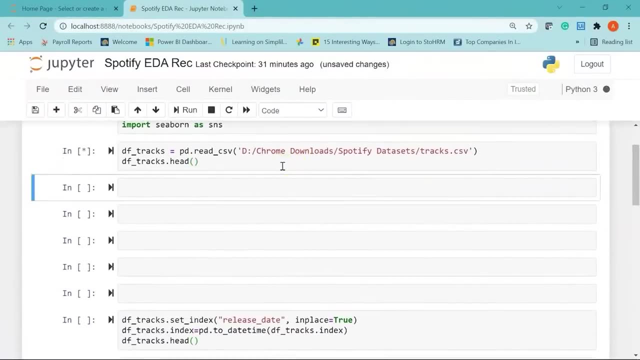 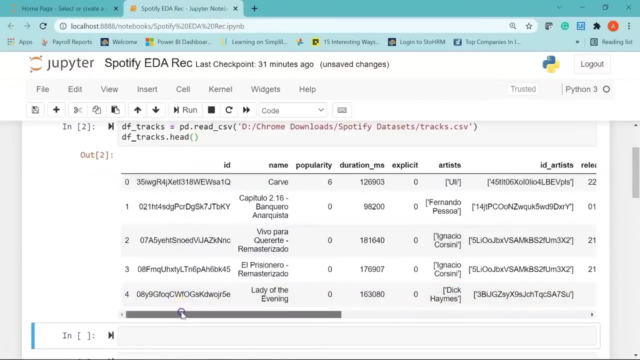 i have a folder called spotify datasets. ok, so let's import and check the first 5 rows in the dataset. so for that i have used the head function. there you go, so here you can see, i have my first 5 rows of information from the dataset. 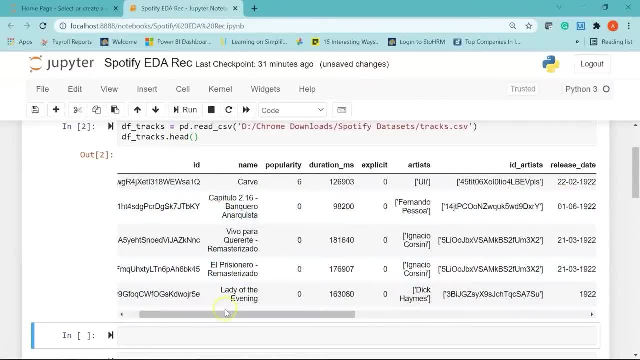 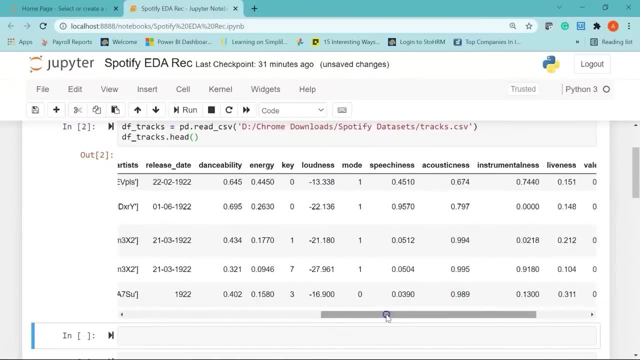 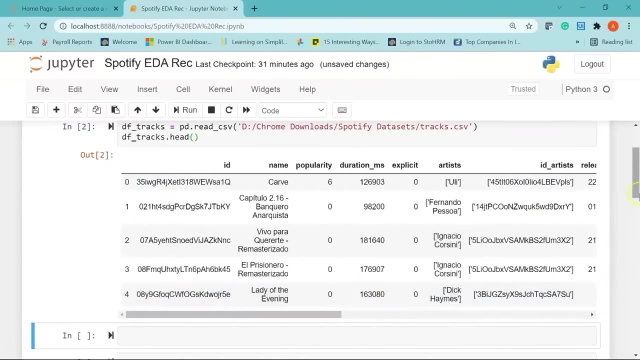 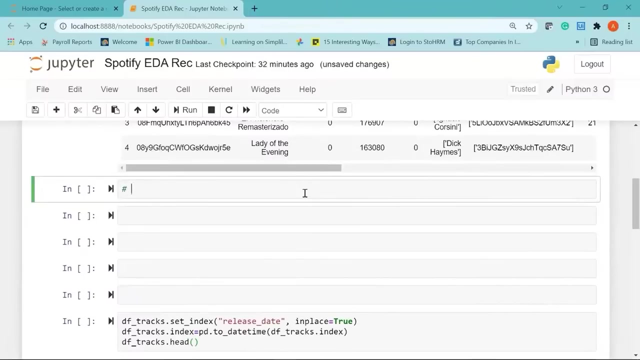 and on the top you can see the different columns. you have id, name, popularity, artist, then we have the release date: danceability, energy key, loudness, liveliness or liveness, valence, tempo and other information. cool, now let's check for null values in the dataset. i'll just give a comment as 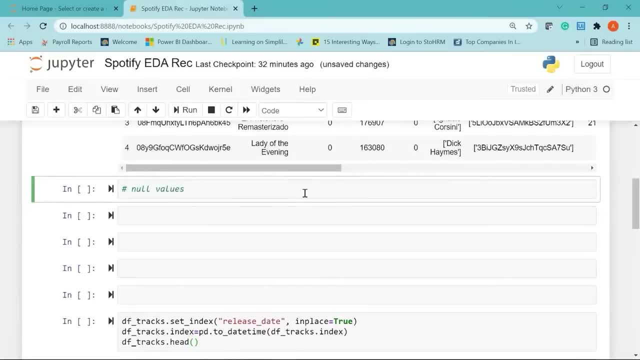 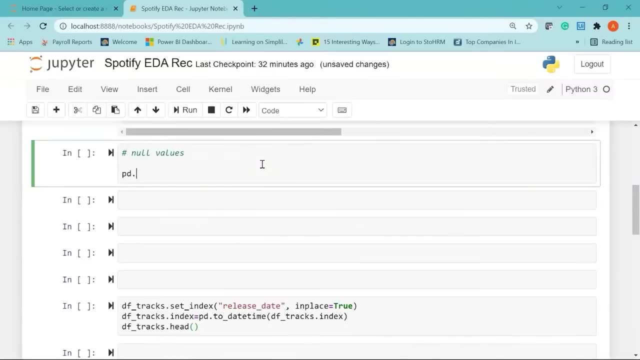 null values. every time when you download a dataset from an open repository, there are chances that the dataset would contain null values, so it's better to check them beforehand. so i am going to use the is null function present in the pandas library pd i am using. 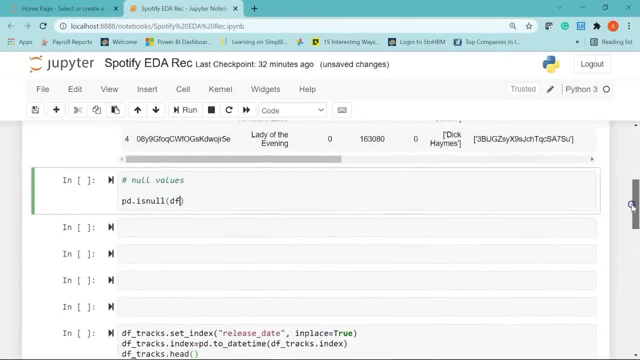 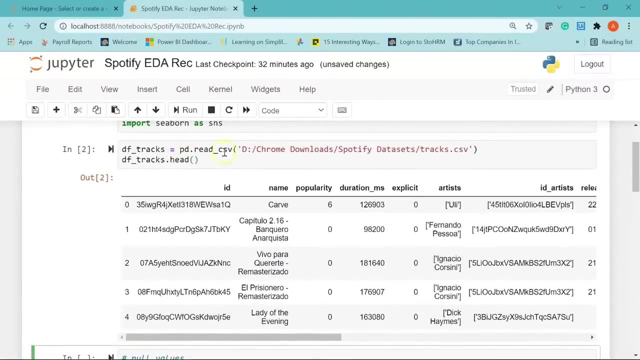 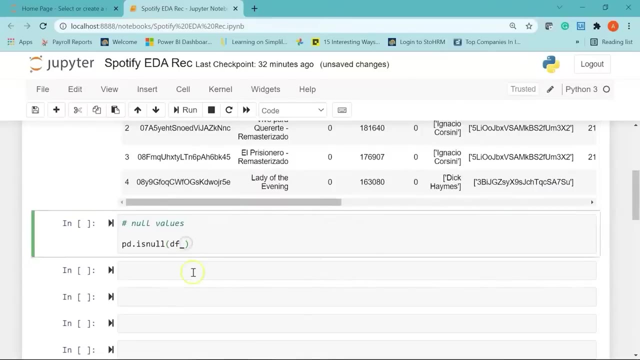 because i had imported pandas as pd, so pd dot is null. then i am going to use the variable name df underscore tracks, because i imported my dataset and stored it in the variable df underscore tracks. so i have my data frame under df underscore tracks variable and then 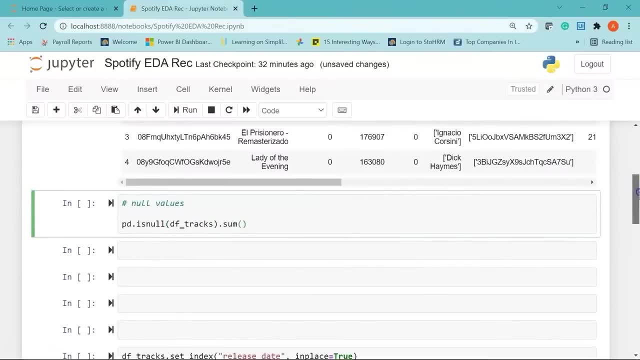 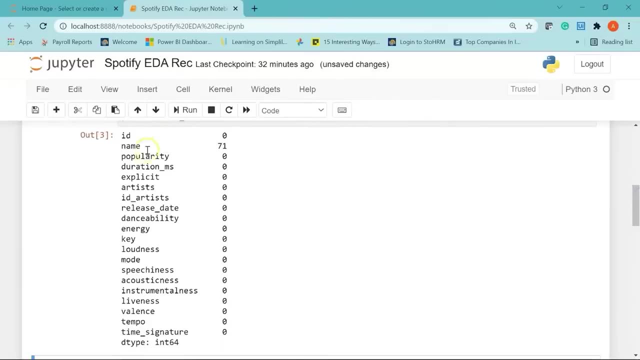 i'll use the sum function to check the total number of null values present in the dataset for each of the columns. if i run it, there you go. so here you can see my name. column has 71 missing values or null values, and we don't have any. 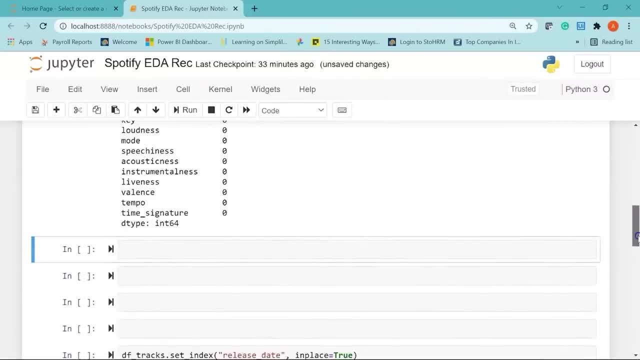 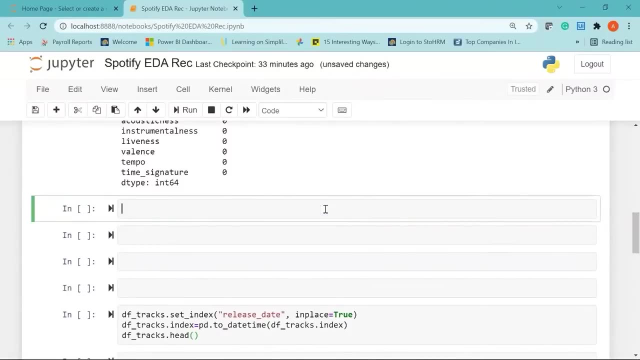 null values for the rest of the columns. okay, now let's use the info method. that will give us the total number of rows and columns in the dataset and we'll also check the data types and the memory usage. so i'll say my data frame name, that is, df, underscore tracks. 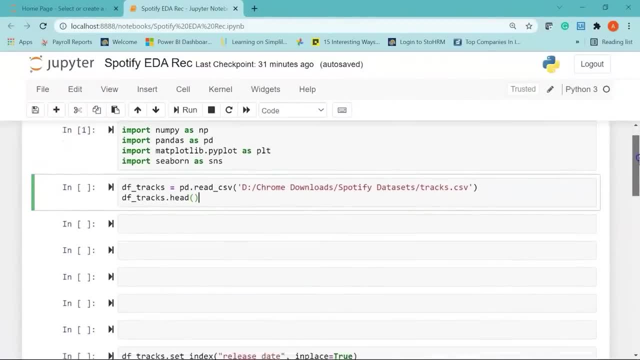 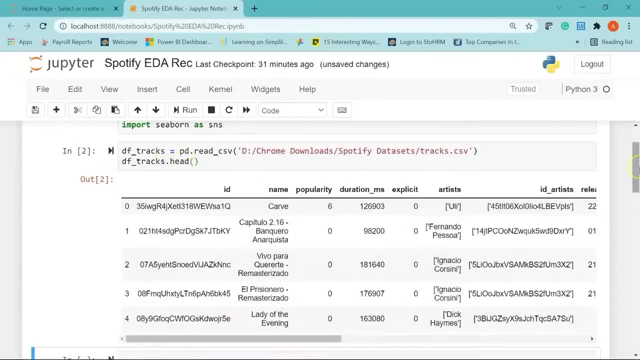 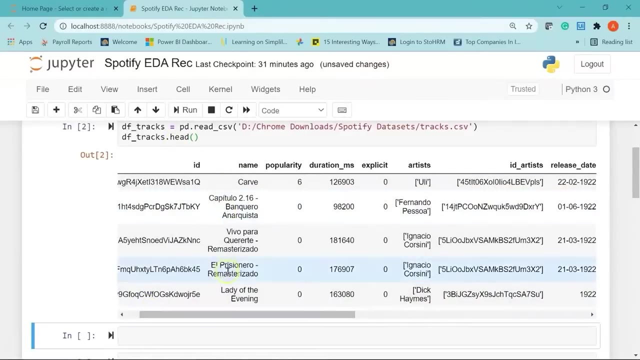 okay, so let's import and check the first five rows in the data set. so for that i have used the head function. there you go, so here you can see. i have my first five rows of information from the data set and on the top you can see the different columns you have: id name, popularity, artist. then 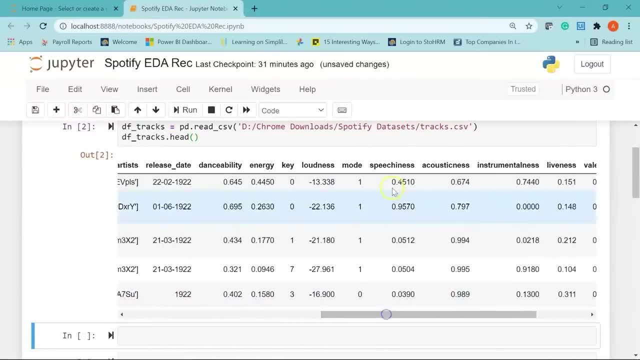 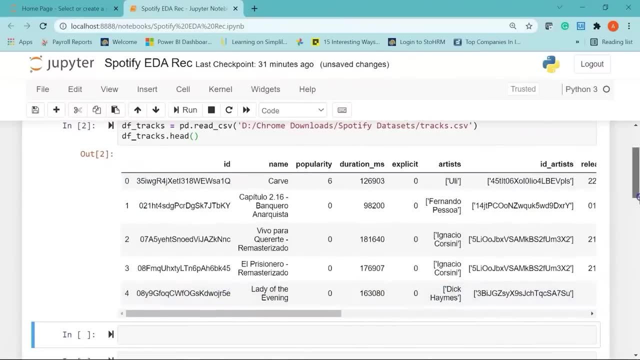 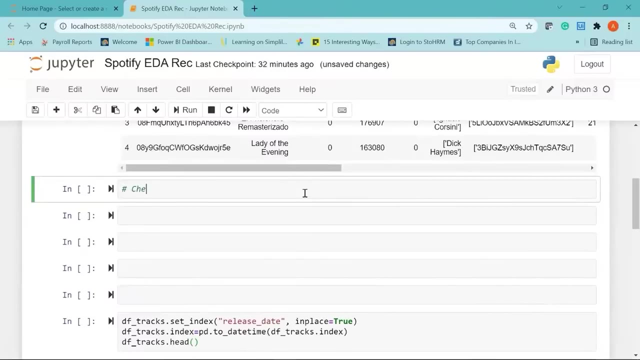 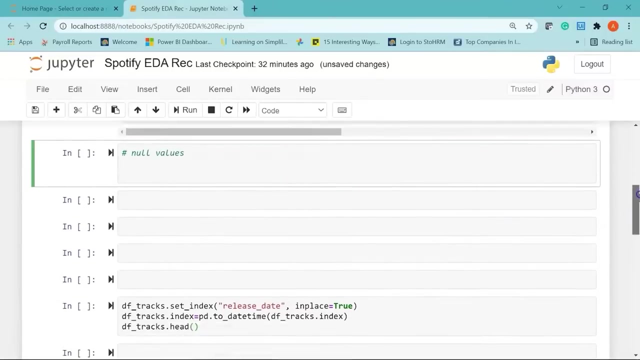 we have the release date: danceability, energy key loudness, liveliness or liveness balance, tempo and other information. cool, now let's check for null values in the data set. i'll just give a comment as null values every time when you download a data set from an open repository. 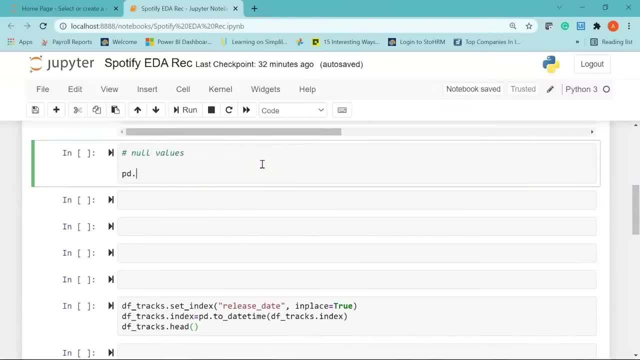 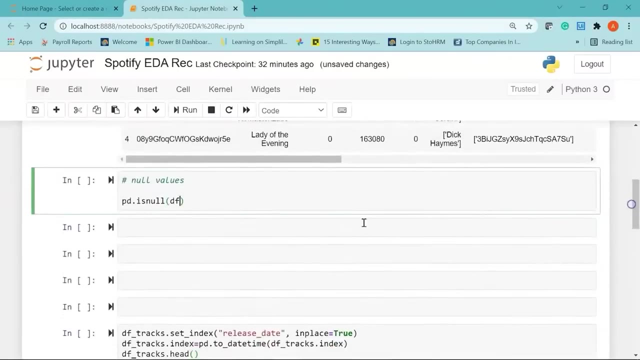 there are chances that the data set would contain null values, so it's better to check them beforehand. so i'm going to use the. is null function present in the pandas library pd i'm using because i had imported pandas as pd, so pd dot is null. then i'm going to use the. 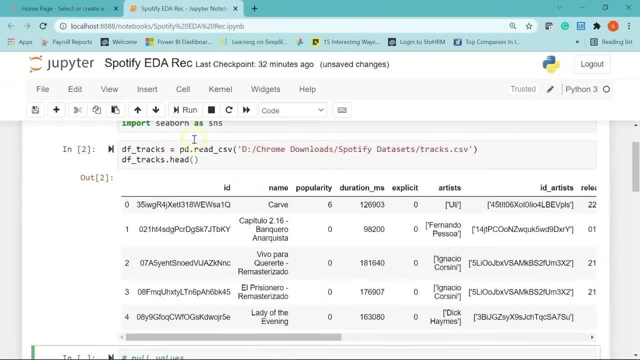 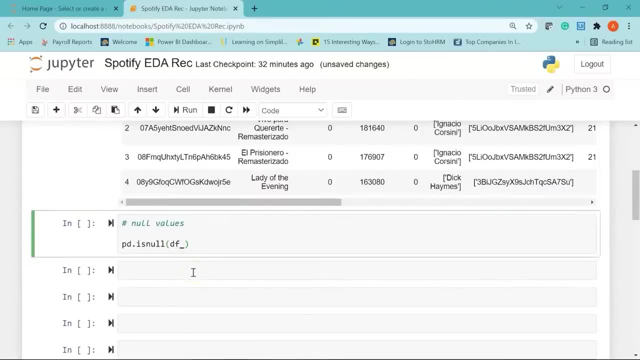 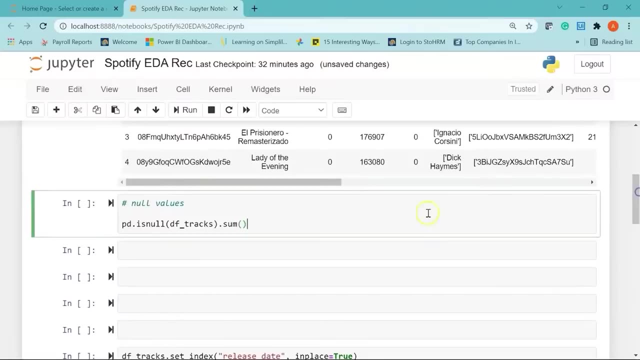 variable name df underscore tracks because i imported my data set and stored it in the variable df underscore tracks. so i have my data frame under df underscore tracks variable and then i'll use the sum function to check the total number of null values present in the data set. for 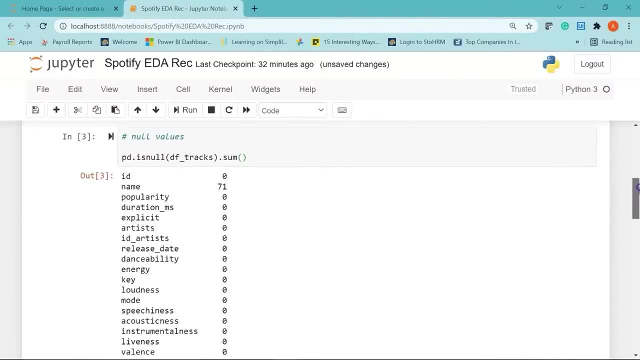 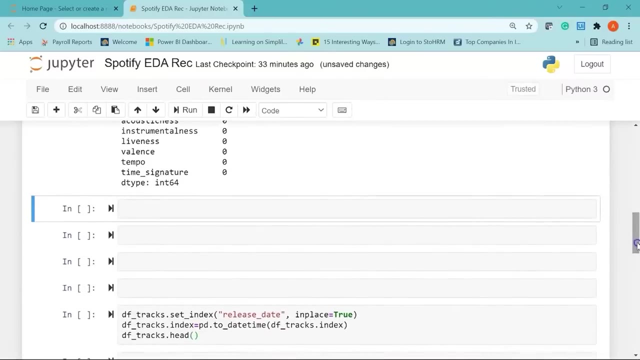 example, if i run it, there you go. so here you can see my name column has 71 missing values or null values, and we don't have any null values for the rest of the columns. okay, now let's use the info method. that will give us the total number of rows and columns in the data set and we'll also check. 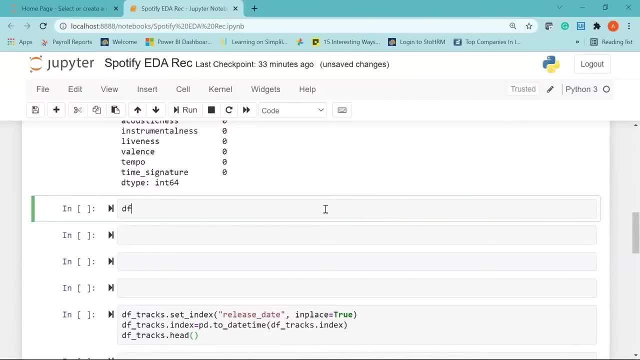 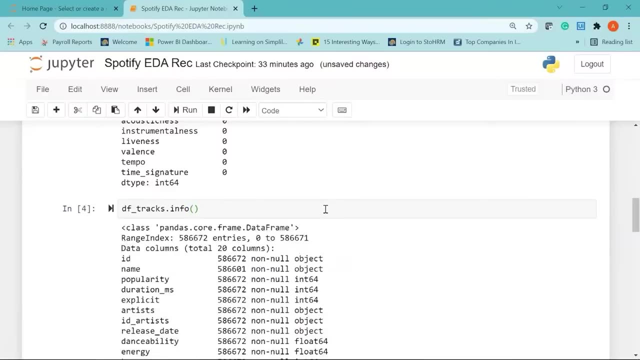 the data types and the memory usage. so i'll say my data frame name, that is df underscore tracks. and we'll also check the data types and the memory usage. so i'll say my data frame name that is df underscore tracks, dot info. if i run it, you can see here. now, if you mark, there are total five. 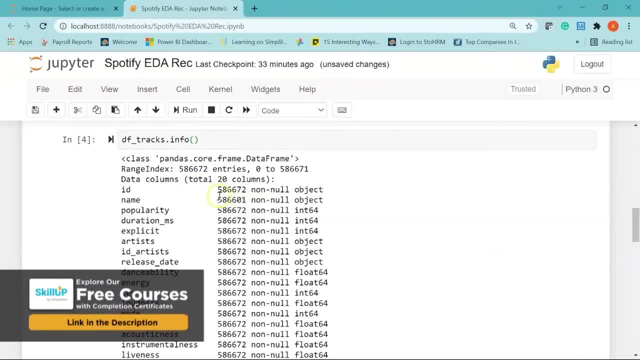 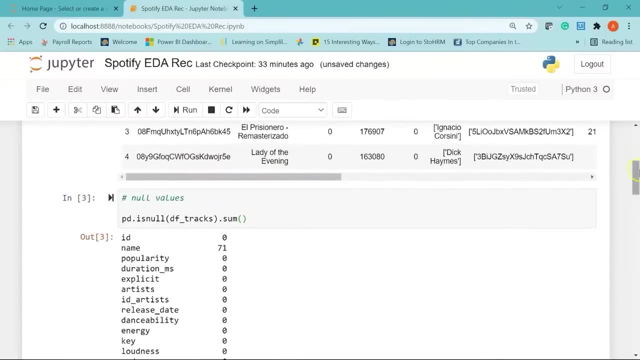 lakh eighty six thousand six hundred and one names or the names of the songs present in the data set, while the rest all have five lakhs eighty six thousand six hundred and seventy two. so clearly, there are total 71 song names or sound tracks missing from our data set. 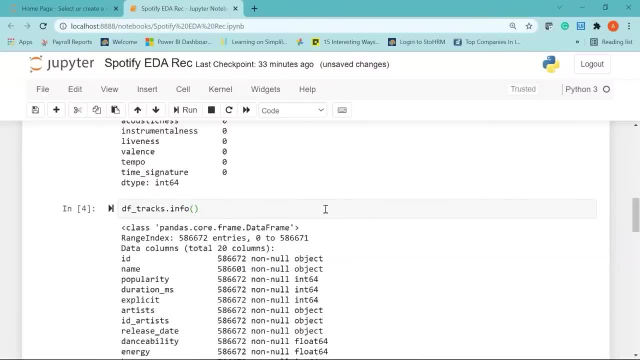 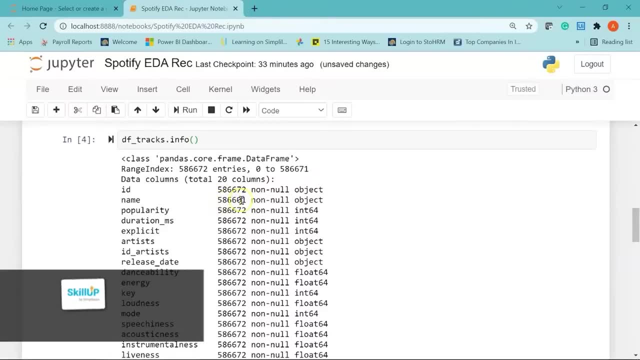 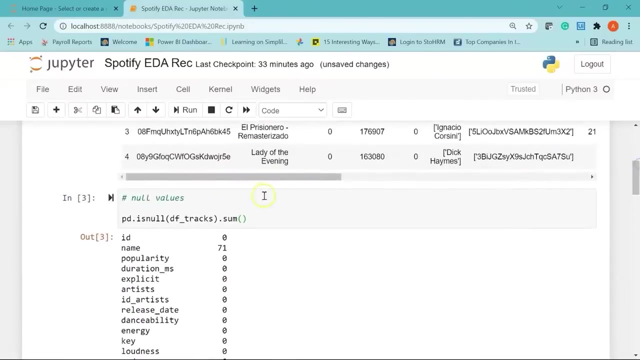 dot info. if i run it, you can see here. now, if you mark, there are total 5,86,601 names or the names of the songs present in the dataset, while the rest all have 5,86,672. so clearly there are total 71 song names or sound. 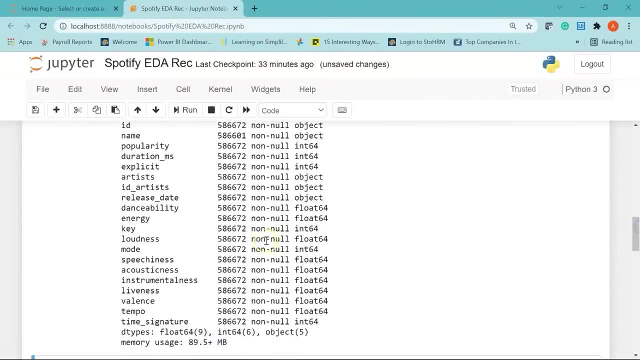 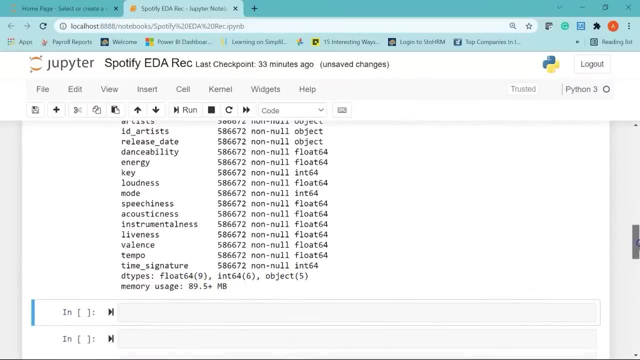 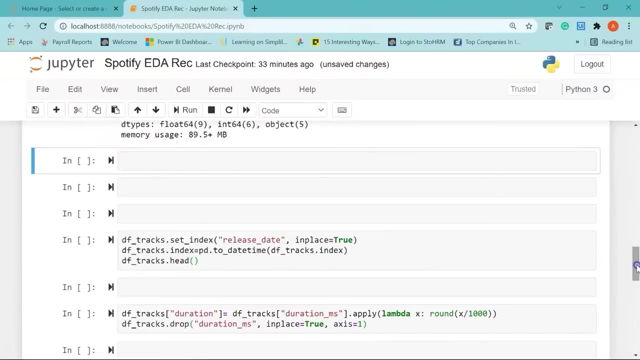 tracks missing from our dataset, and below you can see the data types we have: float, integer and object, and then you can see the memory usage. cool, now, before i move ahead with our next analysis, i have another question for you. which artist or musician has the most number of followers on spotify? 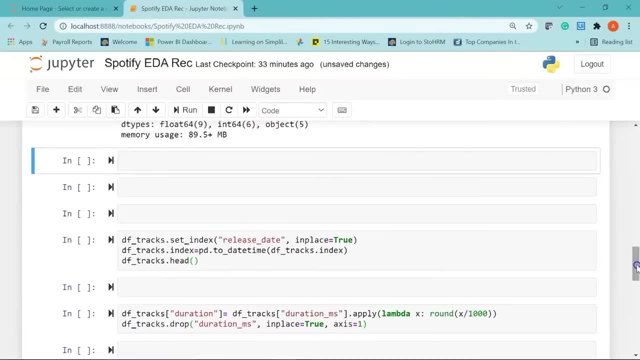 i repeat: which artist or musician has the most number of followers on spotify? please put your answer in the comment section below. we would be happy to hear from you. now. let's move ahead and do our first major analysis. in this demo, we are going to find the 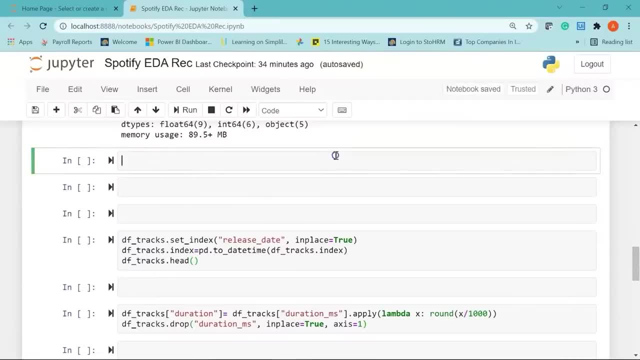 10 least popular songs present in the spotify dataset. so i'll create a variable called sorted underscore, dl. that will be equal to my data frame name, that is df underscore tracks, dot. i'm going to use the sort underscore values function and say my column name is popularity. 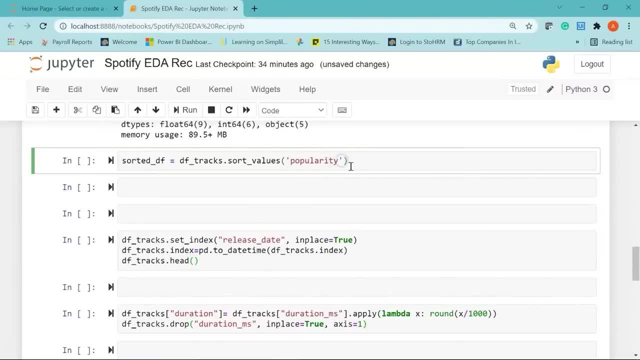 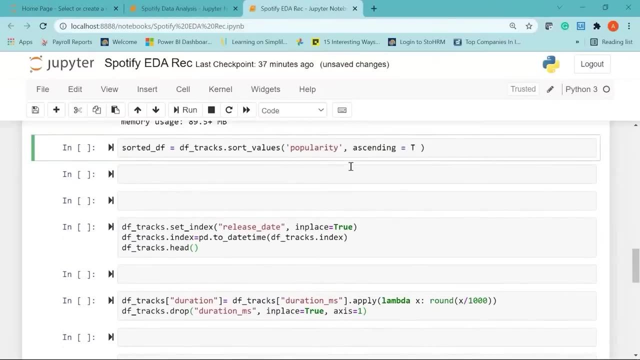 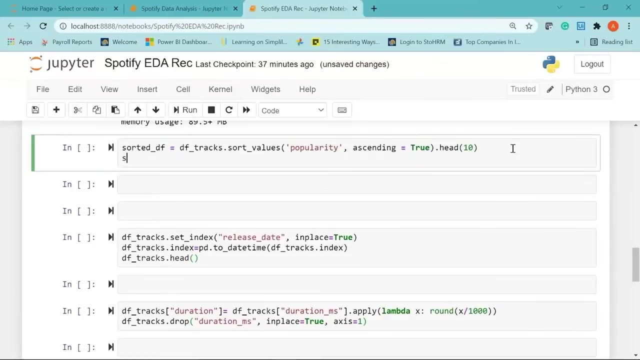 so i'm going to sort the values based on the popularity and then say ascending equal to true, since i want only the least popular songs. and then i'm going to say head of 10, which means i want the top 10 least popular songs. now let's go ahead. 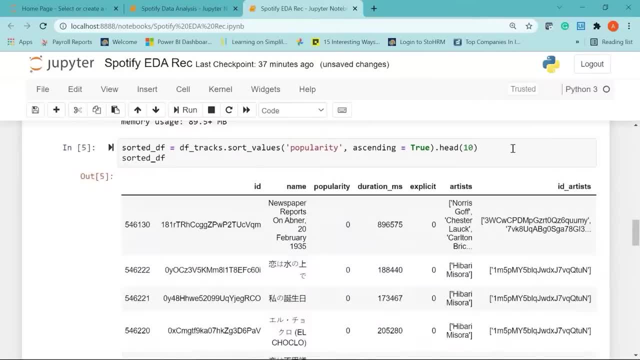 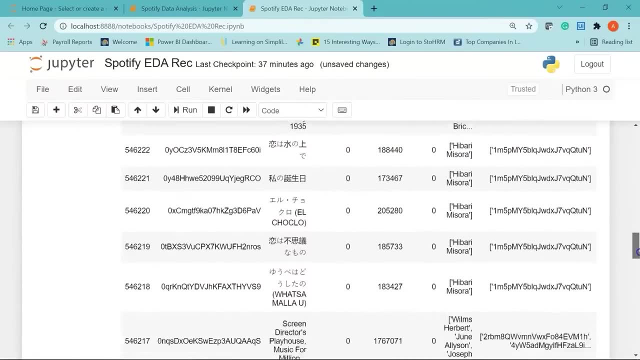 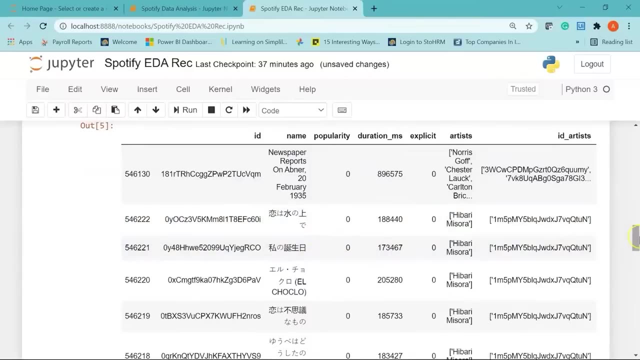 and print sorted underscore dl. if i run it, you can see we have the list of 10 least popular songs on spotify. you can see that the popularity is zero and you can see the names of the songs. some of them are songs which are not in english language. 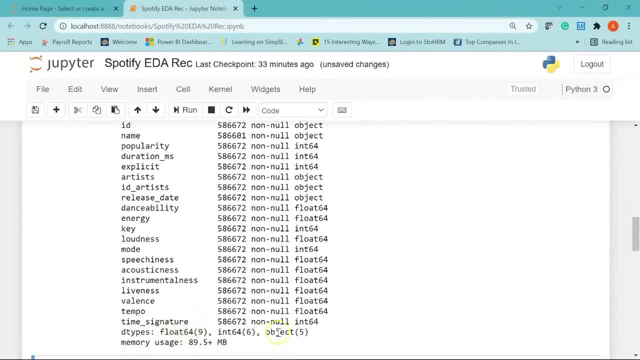 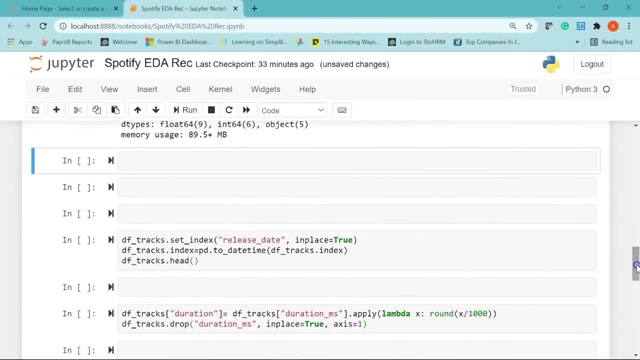 and below you can see the data types we have- float, integer and object- and then you can see the memory usage. cool, now, before i move ahead with our next analysis, i have another question for you: which artist or musician has the most number of followers on spotify? i repeat: which artist or musician has the most number of followers on spotify? 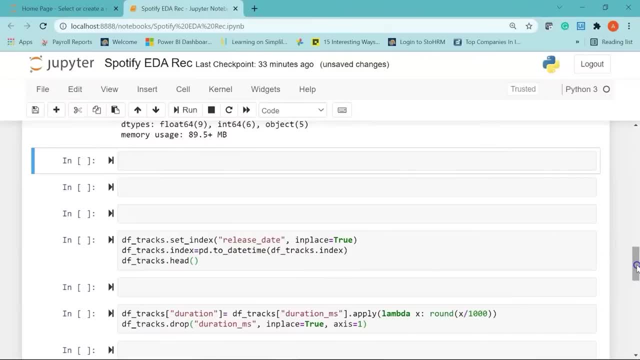 please put your answer in the comment section below. we would be happy to hear from you. now. let's move ahead and do our first major analysis. in this demo we are going to find the 10 least popular songs present in the spotify data set, so i'll create a variable called sorted underscore. 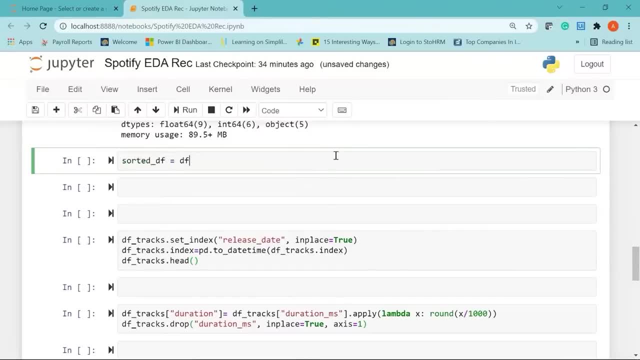 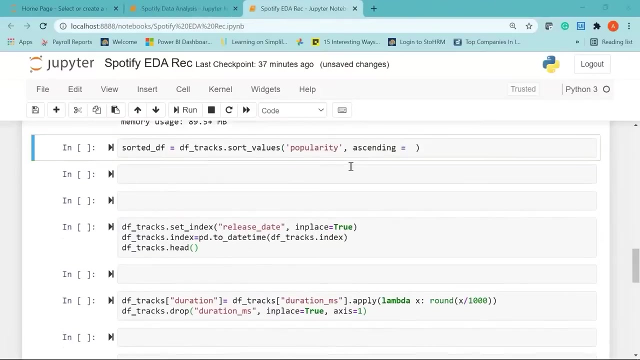 df, that will be equal to my data frame name, that is df. underscore tracks- dot. i'm going to use the sort underscore values function and say my column name is popularity. so i'm going to sort the values based on the popularity and then say: ascending, equal to. 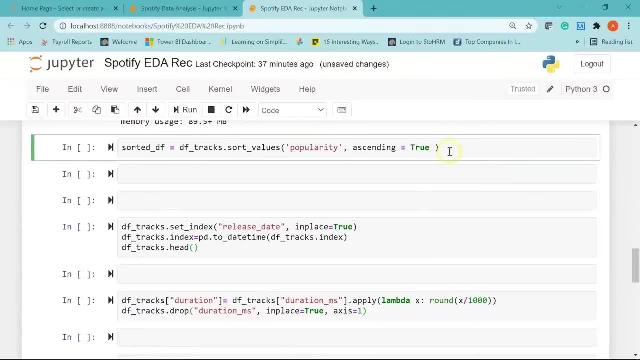 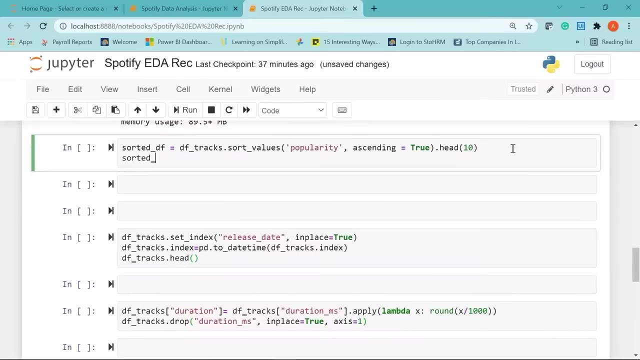 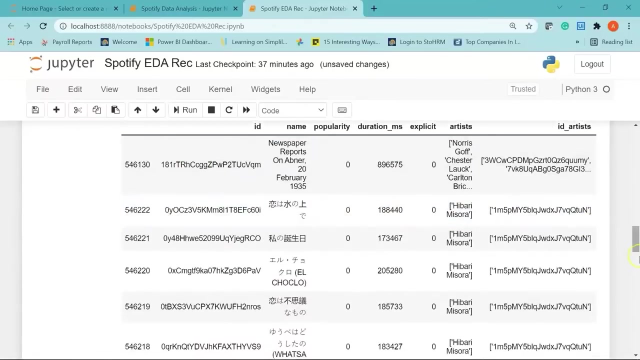 true, since i want only the least popular songs and then i'm going to say head of 10, which means i want the top one, 10 least popular songs. now let's go ahead and print sorted underscore dear. if i run it, you can see we have the list of 10 least popular songs on spotify. you can see the popularity is zero. 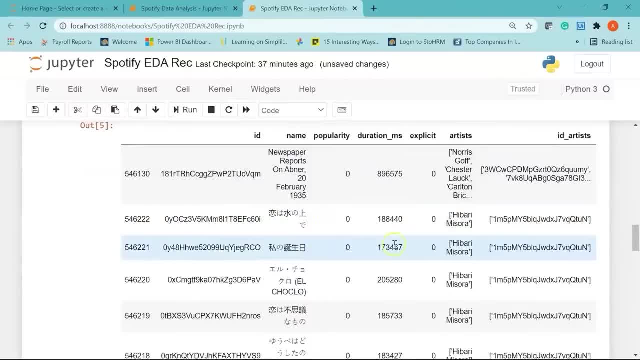 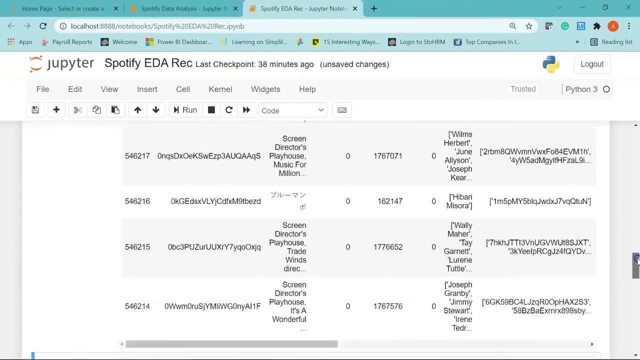 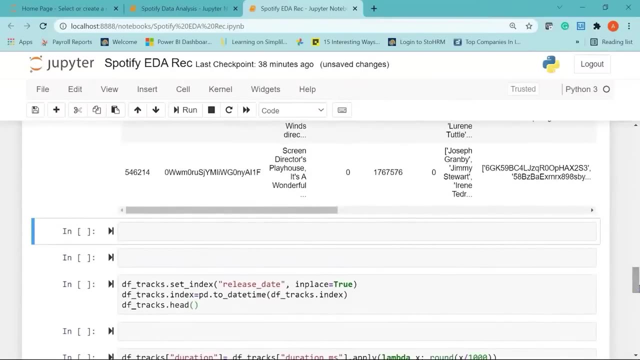 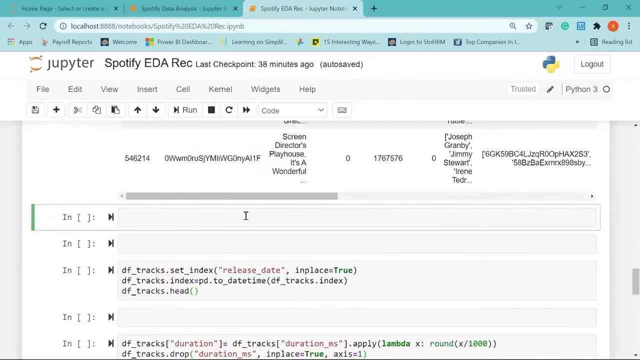 and you can see the names of the songs- some of them are songs which are not in english language- and you can see the artist names as well. cool. now, moving ahead, let's see some descriptive statistics for the numerical variables that are present in our column. so i'll say df, underscore, tracks, dot, describe, which is the function to get some. 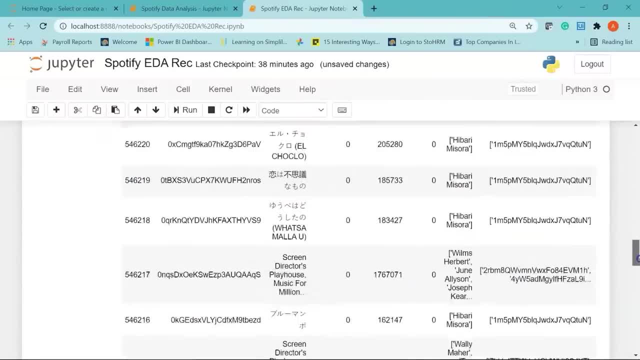 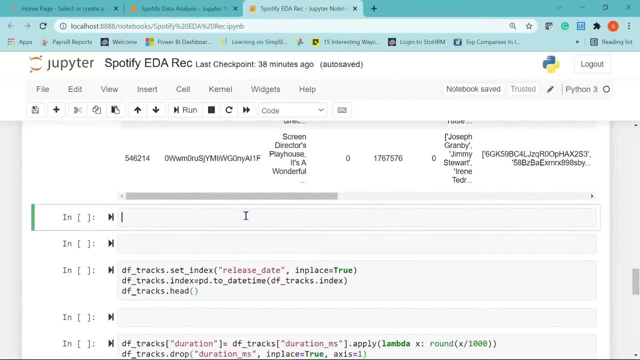 and you can see the artist names as well. cool. now, moving ahead, let's see some descriptive statistics for the numerical variables that are present in our column. so i'll say df, underscore, tracks, dot, describe, which is the function to get some descriptive statistics, and i'm going to use the 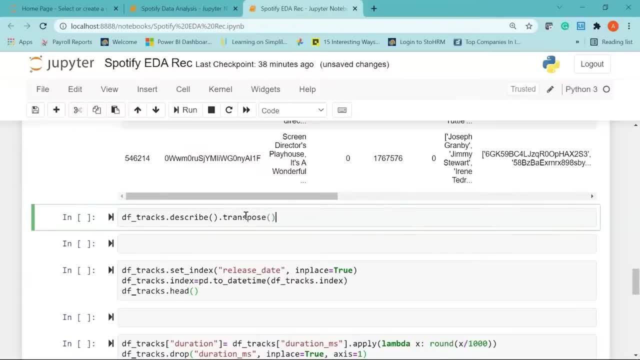 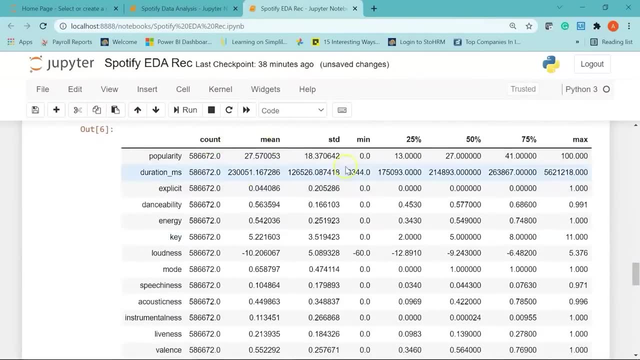 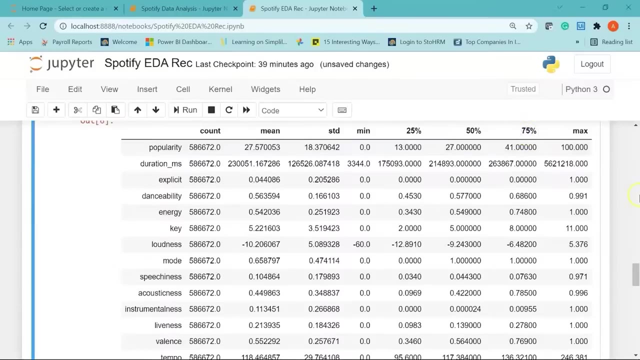 transpose function. after that, if i run it, there you go. so we have the statistics about count, mean, standard deviation, minimum value, 25th percentile, 50th percentile, 75th percentile and the maximum value for these columns like popularity, duration and milliseconds. then we have energy. 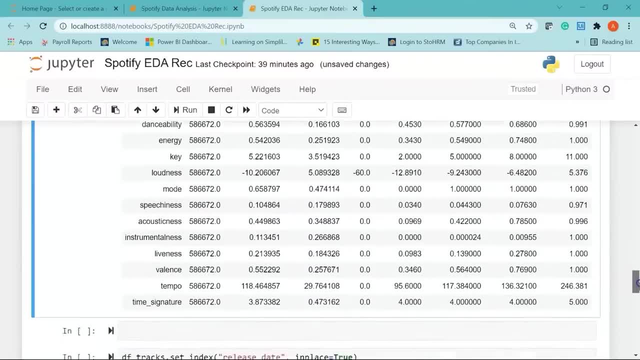 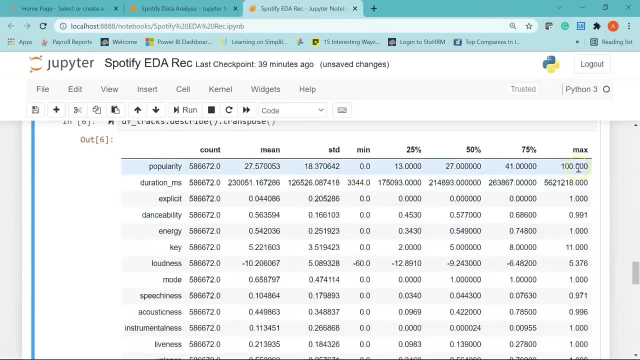 key loudness mode. cool now if you see this popularity column, the minimum value is zero and the maximum value is 100 and you can see the 50th percentile is 27, which is essentially the median. you have the standard deviation as 18.37. 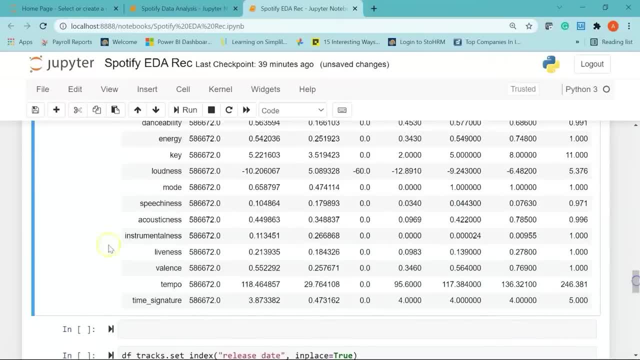 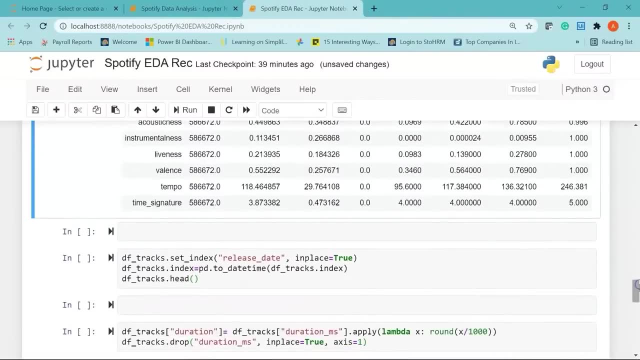 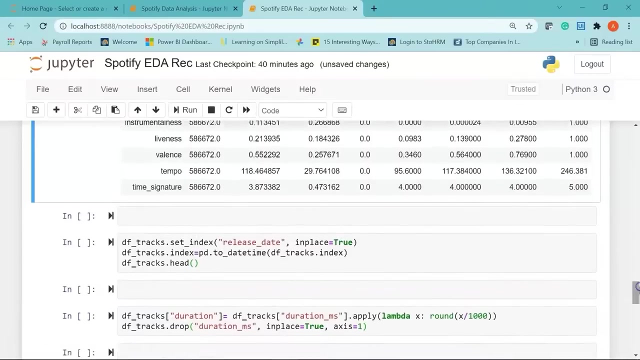 then, similarly, you can check for the other features as well. cool, now we'll see the 10 most popular songs which are greater than 90. so we are going to check for the top 10 songs with popularity greater than 90. let me show you how to do it. 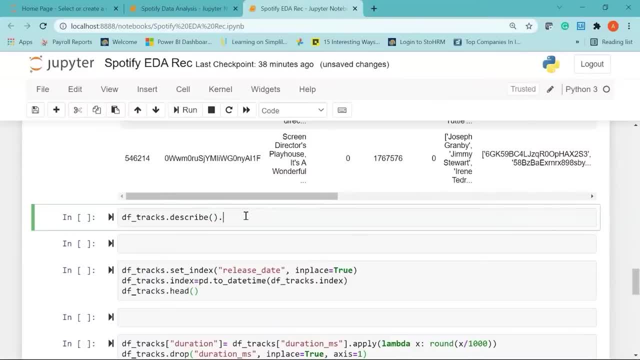 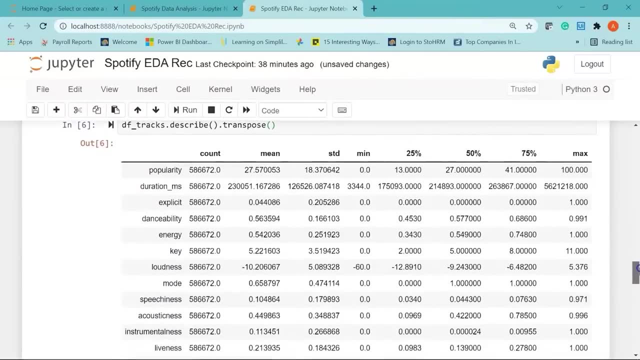 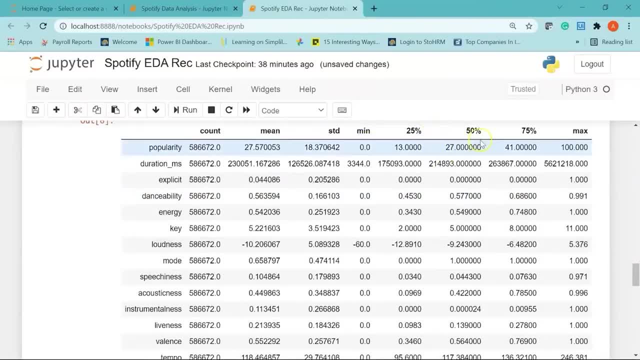 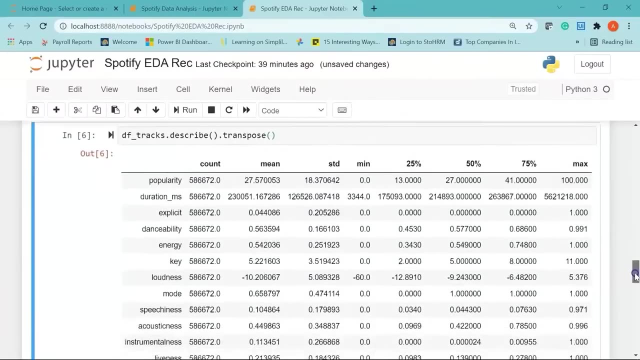 minimum value- 25th percentile, 50th percentile, 75th percentile- and the maximum value for these columns like popularity duration in milliseconds. then we have energy key loudness mode- cool now if you see this popularity column, the minimum value is zero and the maximum value is: 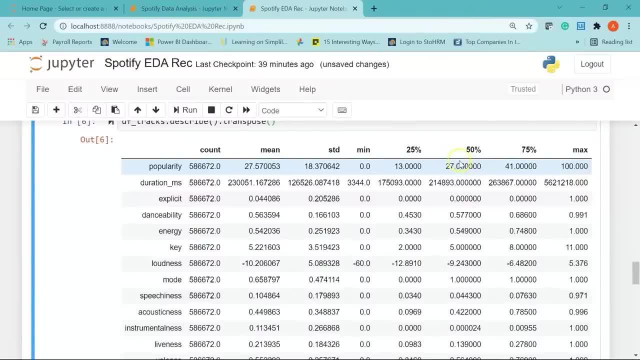 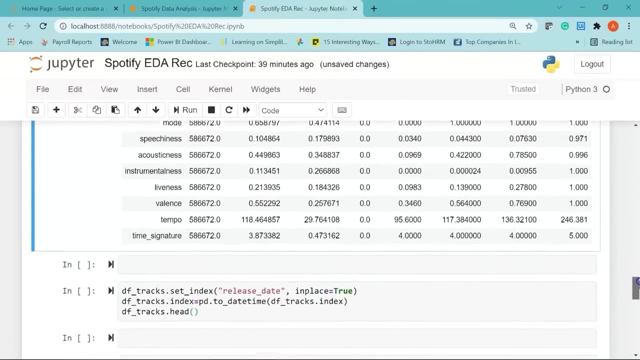 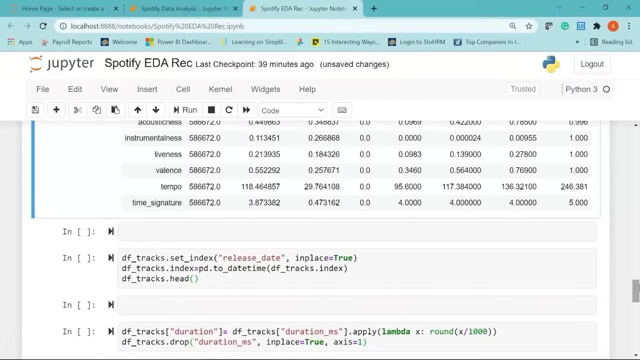 100 and you can see the 50th percentile is 27, which is essentially the median. you have the standard deviation as 18.37. then, similarly, you can check for the other features as well. cool, now we'll see the 10 most popular songs which are greater than 90. so we are going to check for the top 10 songs. 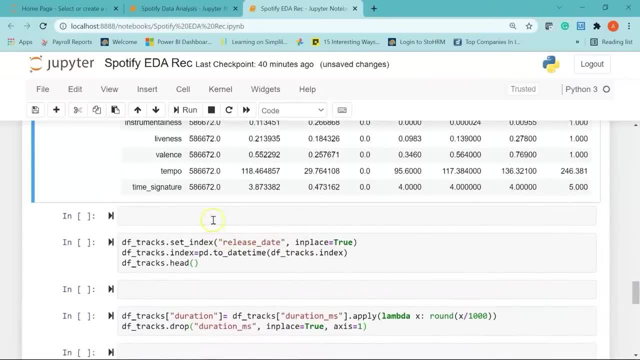 with popularity greater than 90. let me show you how to do it. so in this cell i am going to create a new variable called most popular, and i'll say df, underscore tracks, dot. this time i'm going to use the query function that is part of panel. 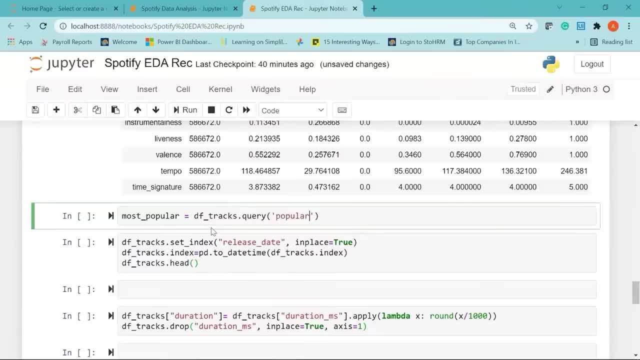 and as library, again, i'll use the column that is popularity, and we'll set the condition: popularity should be greater than 90. i'll give a comma and say in place equal to false, because i don't want to change my original data frame, and then i'll say sort underscore values. 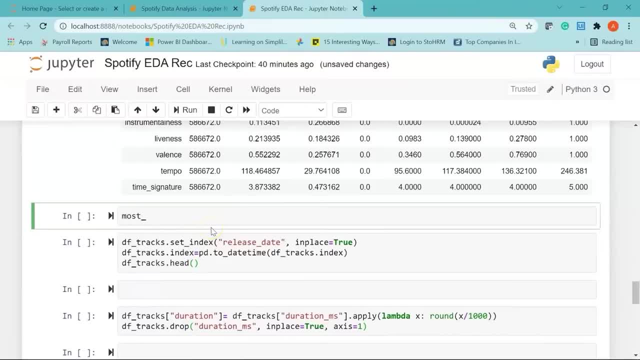 so in this cell i am going to create a new variable called most popular and i'll say df, underscore, tracks, dot. this time i'm going to use the query function that is part of pandas library. again, i'll use the column that is popularity and we'll set the condition. 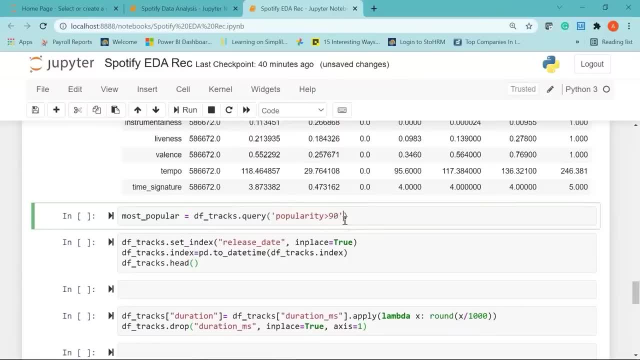 popularity should be greater than 90. i'll give a comma and say in place equal to false, because i don't want to change my original data frame. and then i'll say sort underscore values and i'm going to sort it based on popularity in descending order. 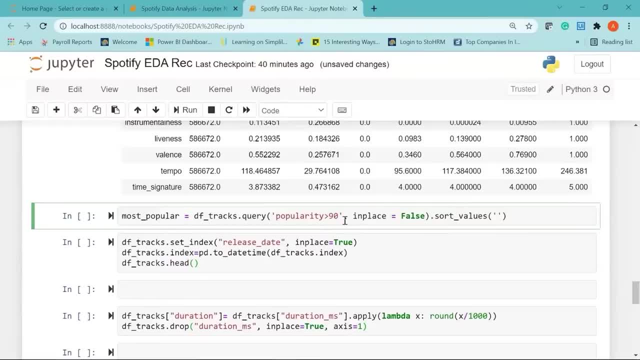 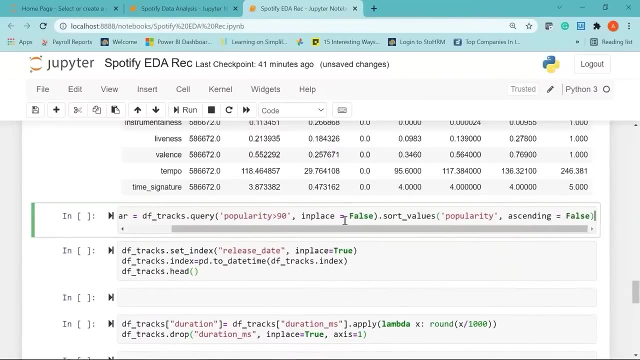 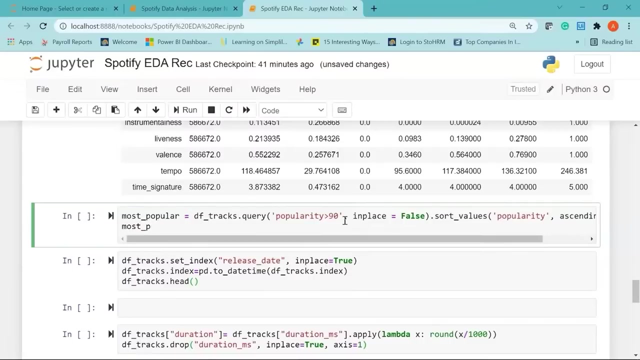 and i'm going to sort it based on popularity in descending order. so i'll say: ascending equal to false, and then let's take only the top 10 popular songs, so i'll say: most popular, use square brackets, use square brackets, and we'll then pass these. 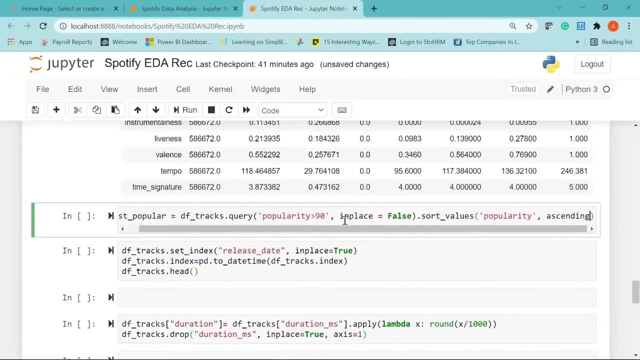 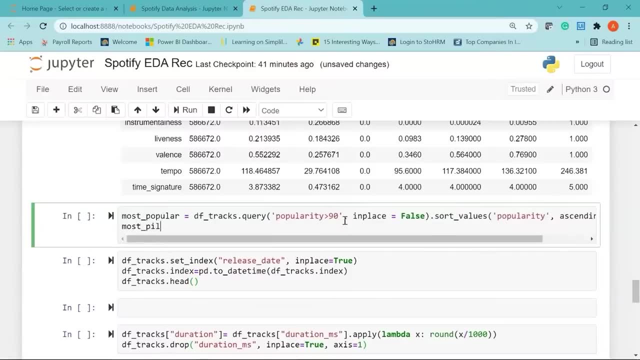 so i'll say: ascending equal to false. and then let's take only the top 10 popular songs. so i'll say: most popular, use square brackets. use square brackets. and we'll then pass the slicing operator and say: colon 10. now, if i run this, there you go. 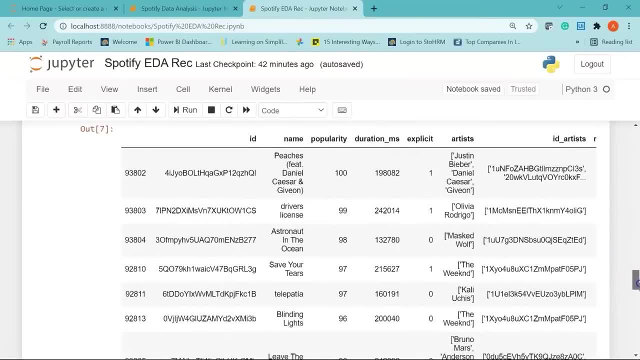 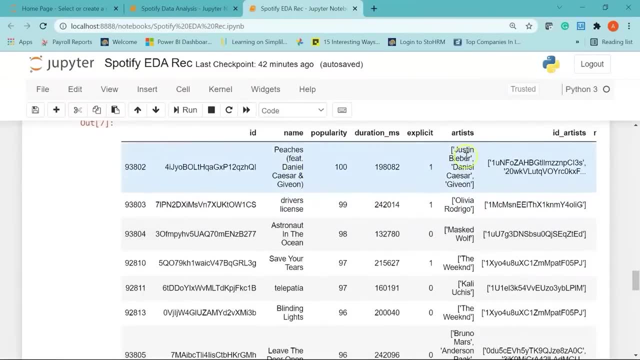 so here you can see the 10 most popular songs that is present in our spotify data set. first we have peaches by justin bieber, daniel cesar and give on. then we also have a song name called driver's license. astronaut in the ocean. 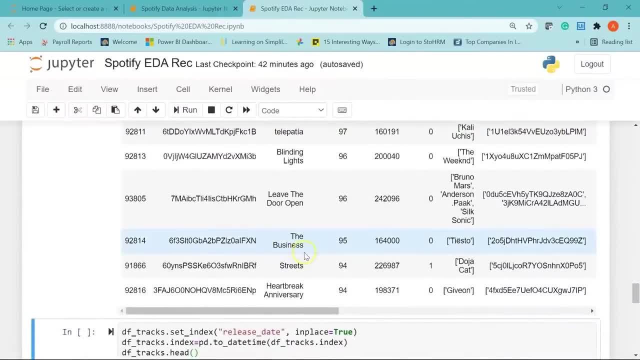 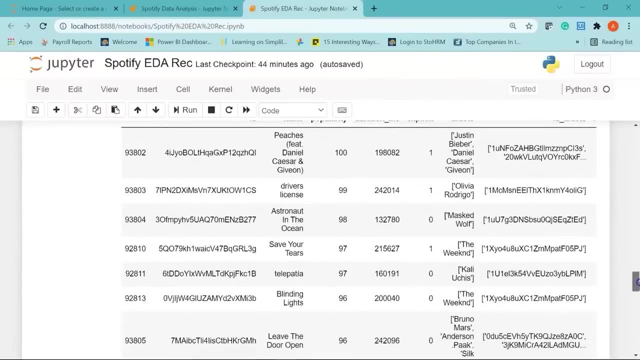 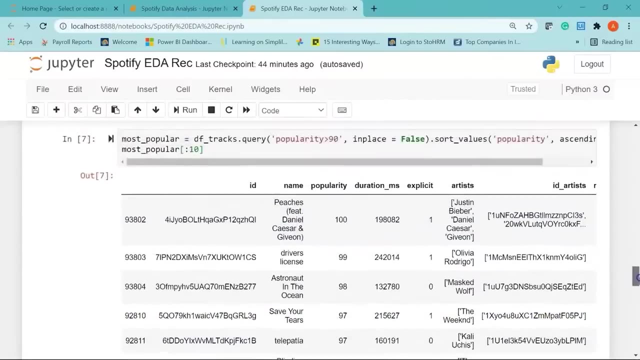 save your tears. we also have the business streets and heartbreak anniversary, so these are the most popular songs that are present in our data set. based on their popularity, you can see peaches has the highest popularity, with 100 all right. now, moving to the next cell. 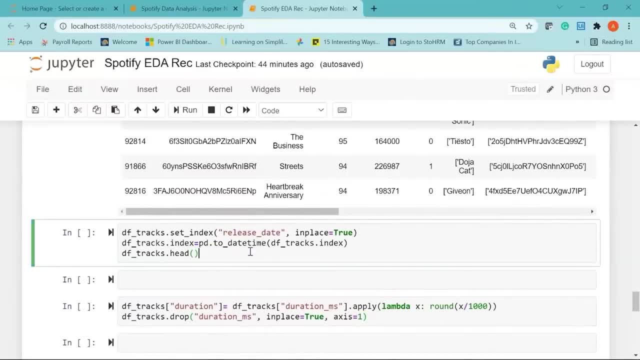 so here we are going to set the index to be release date column in the main data frame. so i am setting my index using the set underscore index function. i have passed in my column name as release date and i'm saying in place equal to true, which means i want to change. 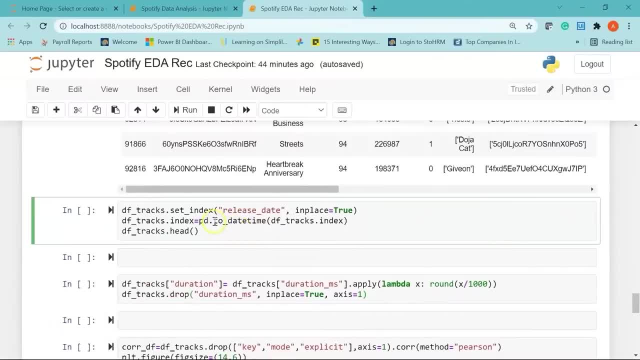 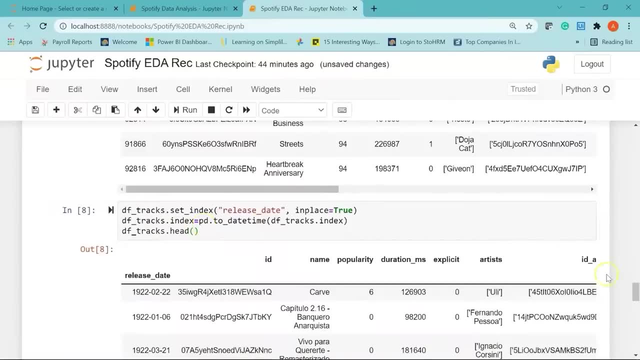 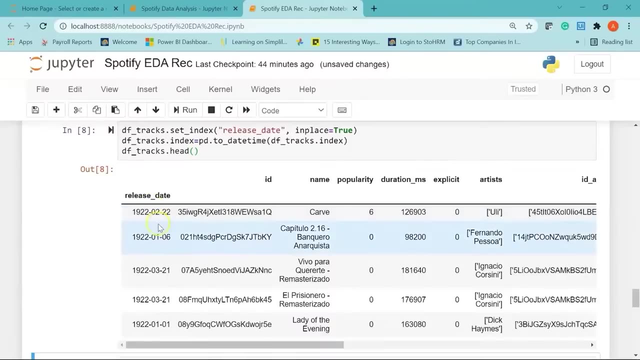 it in my original data frame and then i'm changing the value to date time format and let's print the head of the data set. so you can see here we have successfully changed our index. now here you can see, instead of 0, 1, 2, 3, we have the release date. 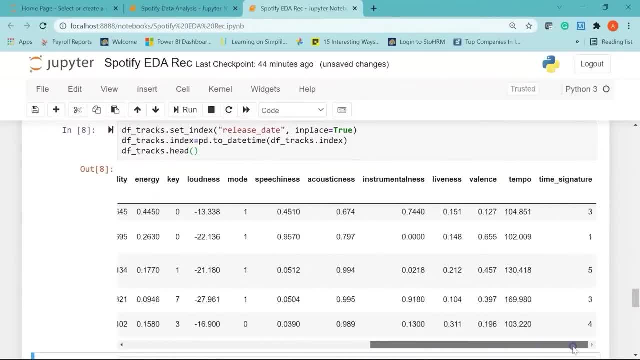 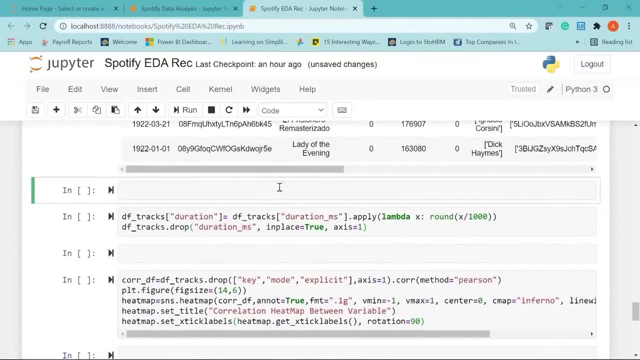 column and the rest of the columns are intact. cool, now let's move ahead. so suppose you want to check the artist at the 18th row in our data set. you can use the index location method for that. let me show you how to filter only specific rows of information. 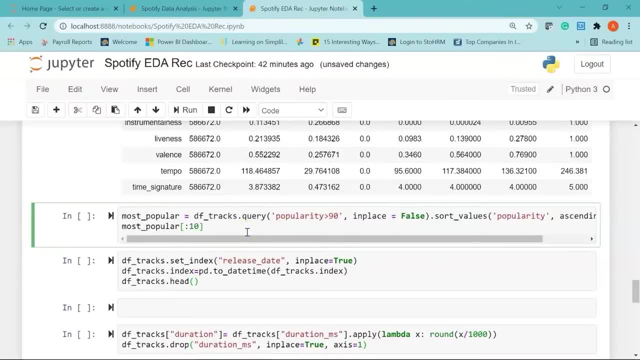 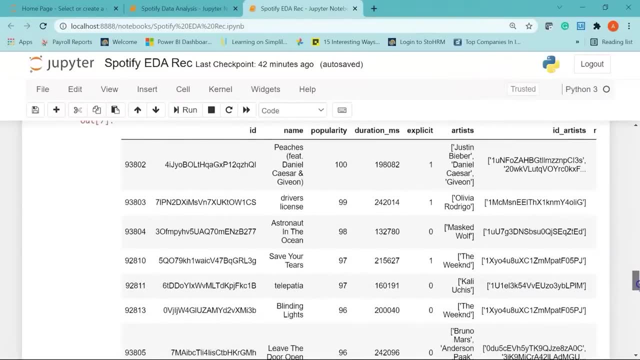 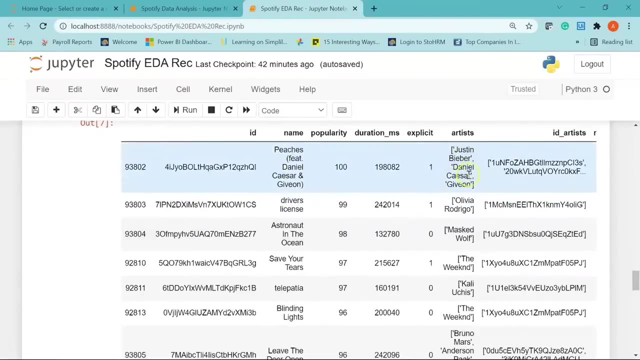 slicing operator and say colon 10. now, if i run this, there you go. so here you can see the 10 most popular songs that is present in our spotify data set. first we have features by justin bieber, daniel cesar and give on. then we also have a song name called driver's license. astronaut in the ocean. 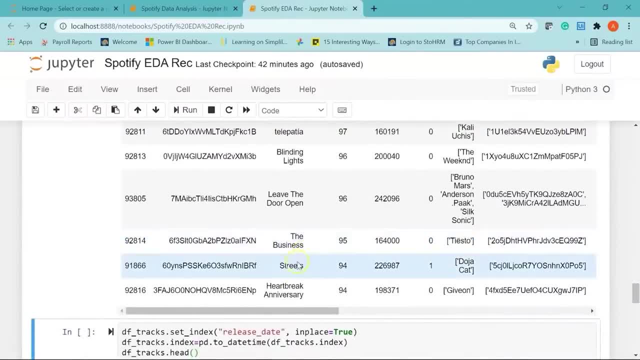 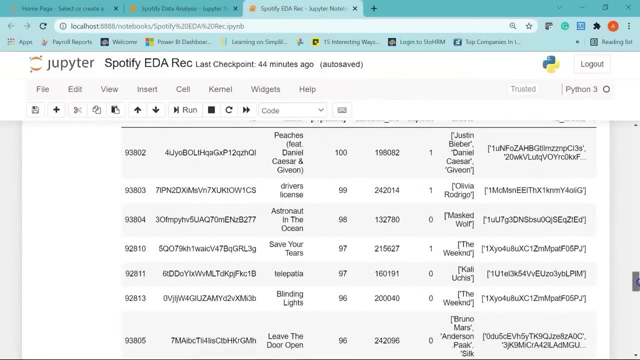 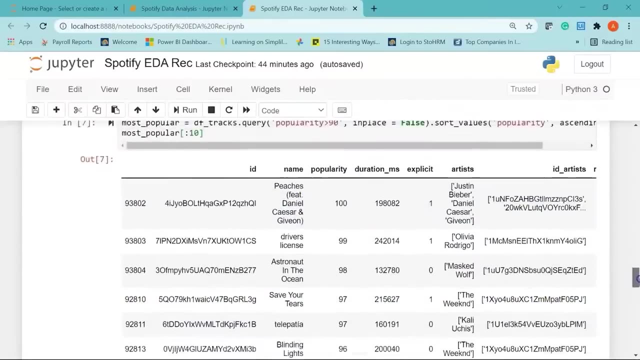 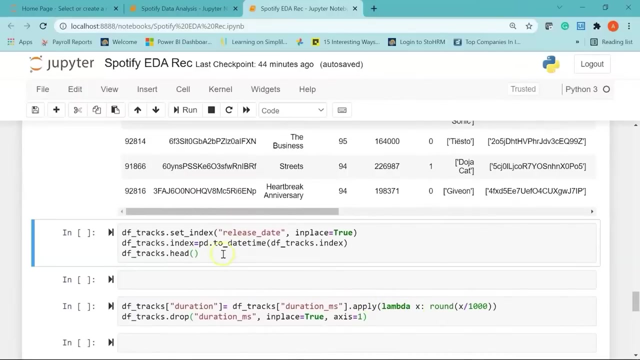 save your tears. we also have the business rates and heartbreak anniversary, so these are the most popular songs that are present in our data set. based on their popularity, you can see peaches has the highest popularity, with 100 all right now moving to the next cell. so here we are going to set the index to be. 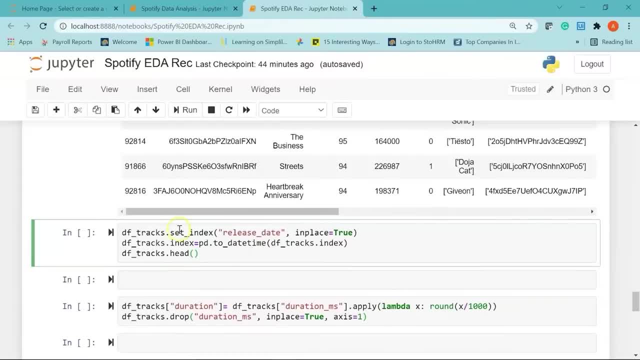 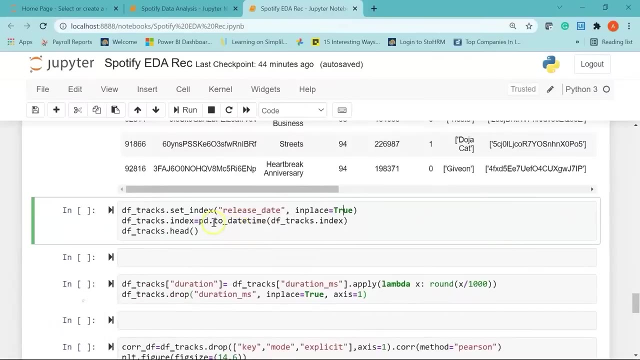 release date column in the main data frame. so i am setting my index using the set underscore index function. i have passed in my column name as release date and i'm saying in place equal to true, which means i want to change it in my original data frame, and then i'm changing the value to date time format. 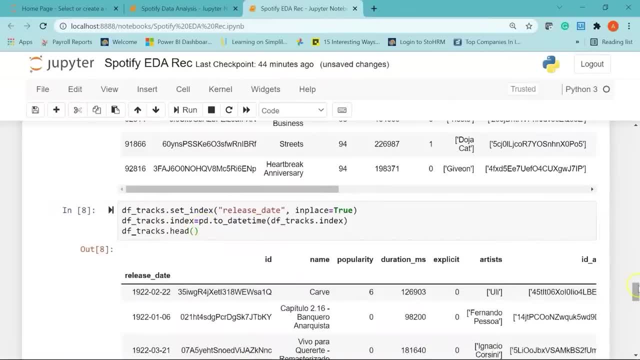 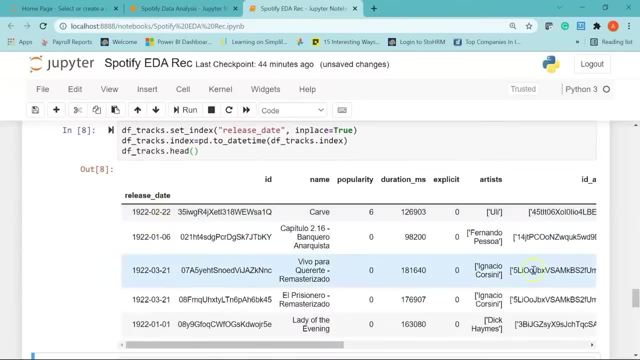 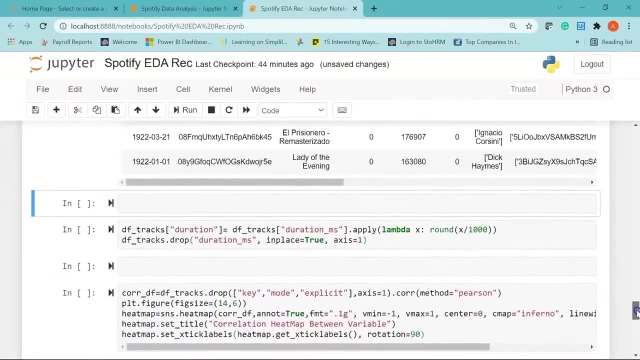 and let's print the head of the data set so you can see: here we have successfully changed our index. now, here you can see: instead of 0, 1, 2, 3, we have the release date column, and the rest of the columns are intact. cool, now let's move ahead. so suppose you want to check the artist at the 18th row in our data set. 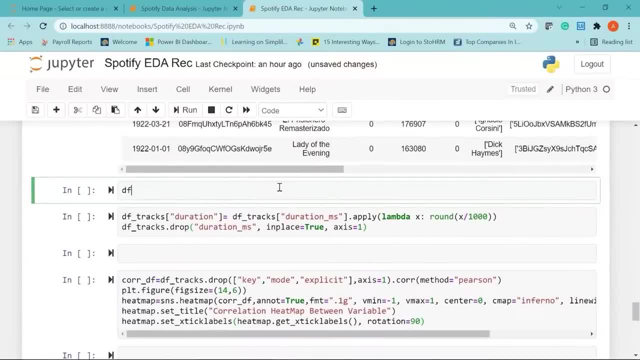 you can use the index location method for that. let me show you how to filter only specific rows of information from the data set. i'll use my data frame df, underscore tracks and, using double square brackets, i'll say my column name, which is artist, and i'll use the column name which is artist and i'll use the. 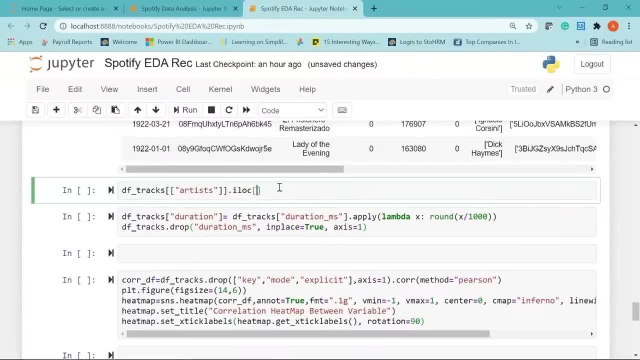 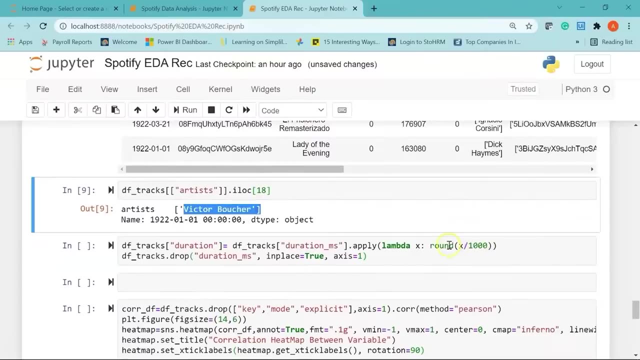 index location method and see, let's say, i want to check the artist who is present in the 18th row in my data set, so i use ilog18. if i run it, the artist name is victor voucher. cool, now let's move ahead. we are going to convert the duration in milliseconds to just seconds, so 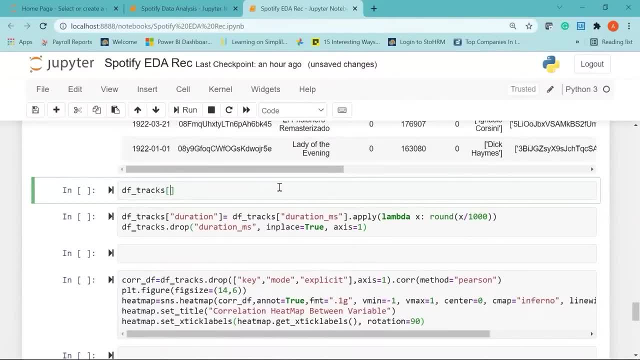 from the data set. i'll use my data frame, df, underscore tracks and, using double square brackets, i'll say my column name, but which is artist, and i'll use the index location method and say, let's say, i want to check the artist who is present in the 18th row in my data set. 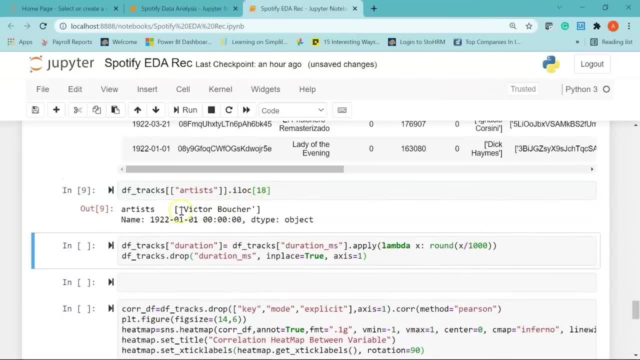 so i'll use iloc 18 if i run it, the artist name is victor boucher. cool, now let's move ahead. we are going to convert the duration in milliseconds to just seconds. so if you see our data set, we have a column called duration in milliseconds. so all our 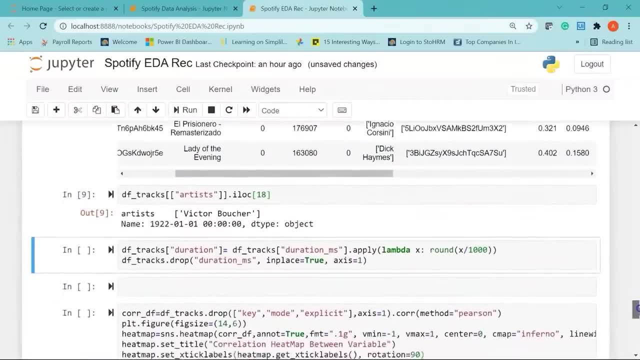 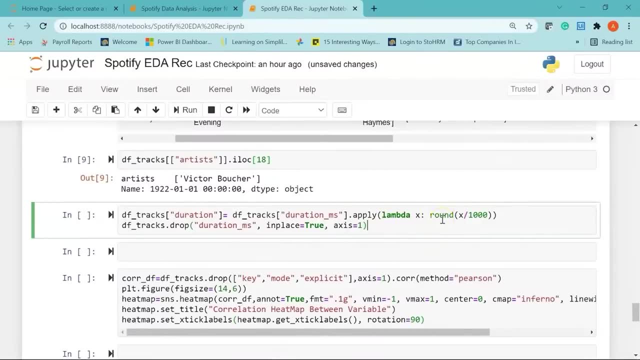 songs are present in milliseconds, let's convert them into just seconds. so for that i'm using the lambda function and dividing the values in milliseconds by thousand so that they get converted into just seconds. i have used in place equal to true, so i want to change it in my original data frame. 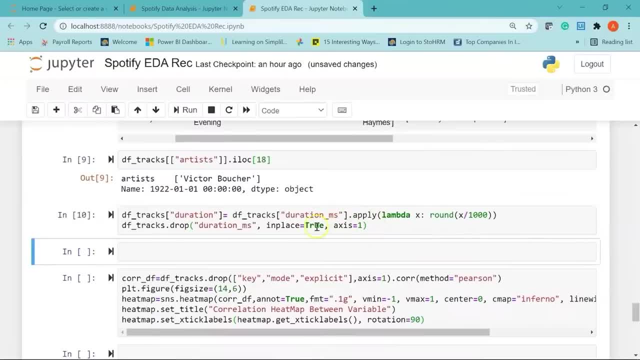 let's run it and do the necessary changes. alright, now we'll print the head of the data set, just to check the duration column. so i'll say df, underscore tracks, dot, duration, dot head. if i run it, there you go. so you can see. the values have now been. 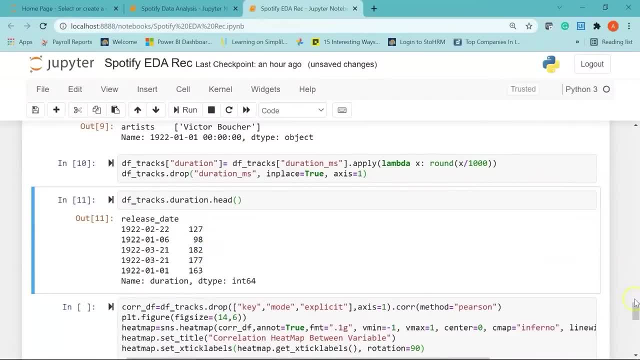 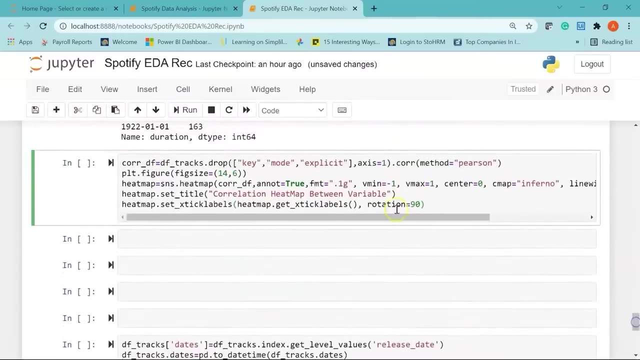 changed to just seconds. cool, i have the final quiz question for you. who has the most monthly listeners on spotify? please put your answers in the comment section below. we'd be glad to hear from you now coming to the next cell. so here we are going to create a first. 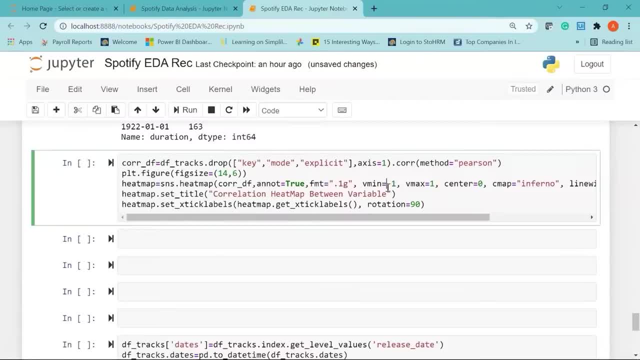 visualization. that is going to be a correlation map. we are going to drop three unwanted columns and those are key, mode and explicit, and then we are going to apply pearson correlation method. now i have set my figure size to 14 comma 6, and then we are using the seaborn. 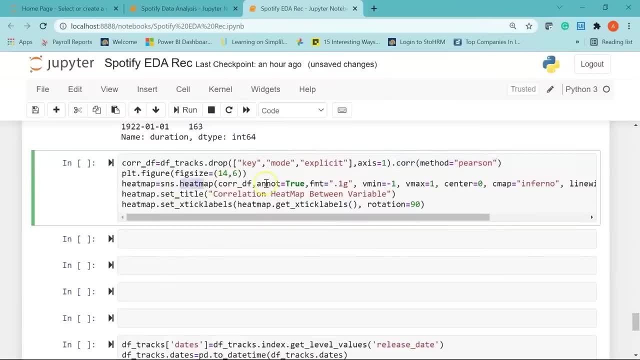 heatmap function to create our correlation map. i have put the variable, that is correlation, underscore df. you can see above we had created this and then i am setting annotation equal to true, so this will write the data value in each cell. i have set fmt equal to dot 1. 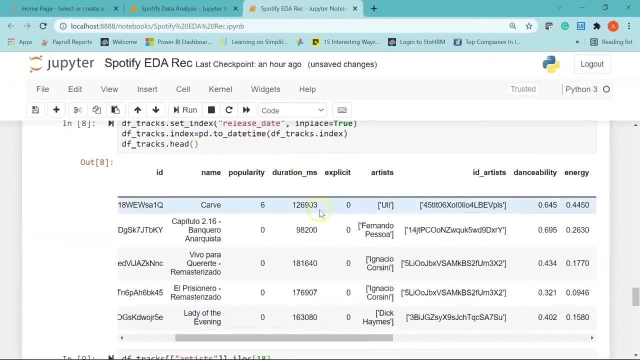 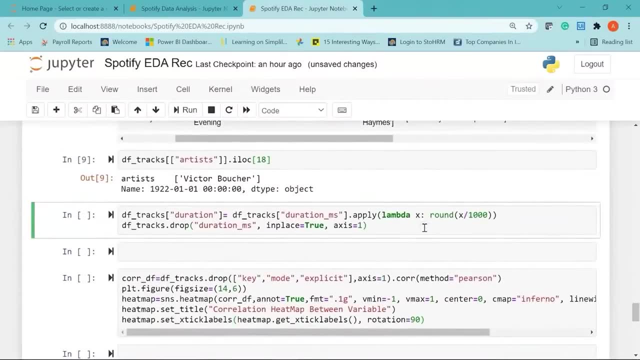 if you see our data set, we have a column called duration in milliseconds, so all our songs are present in milliseconds. let's convert them into just seconds. so for that i'm using the lambda function and dividing the values in milliseconds by thousand so that they get converted into just seconds. i have used in 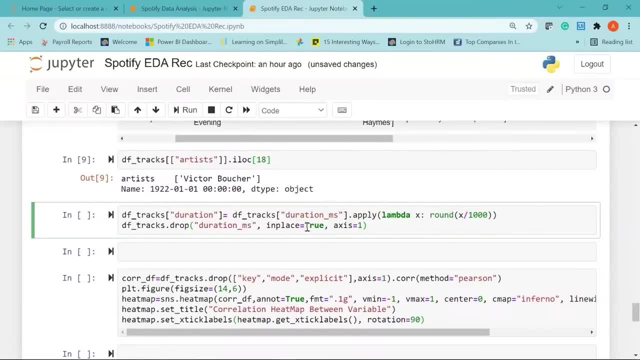 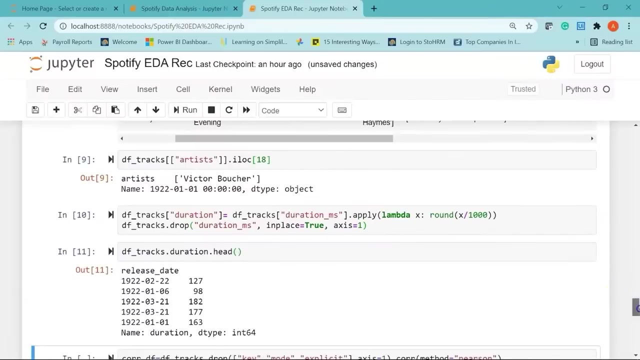 place equal to true. so i want to change it in my original data frame. let's run it and do the necessary changes. all right, now we'll print the head of the data set, just to check the duration column. so i'll say df underscore tracks, dot, duration, dot head. if i run it, there you go so. 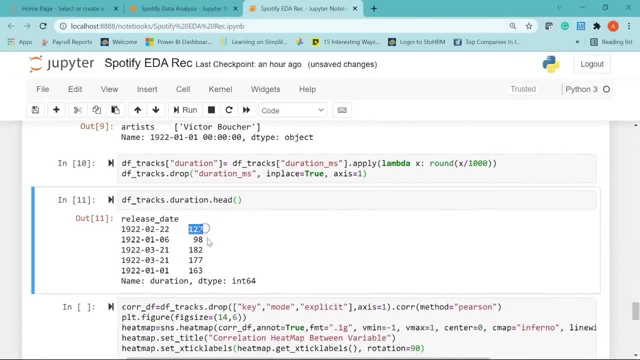 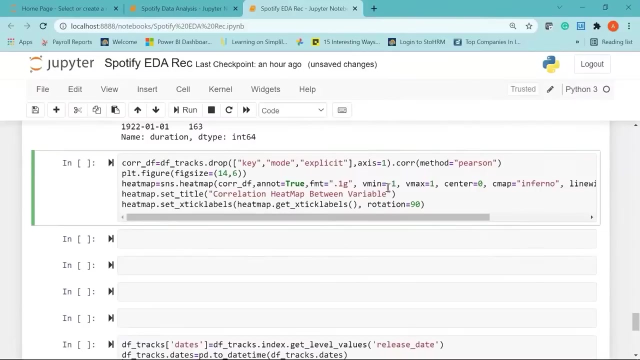 you can see the values have now been changed to just seconds. cool, i have the final quiz question for you. you who has the most monthly listeners on spotify. please put your answers in the comment section below. we'd be glad to hear from you. now coming to the next cell. so here we are going to create. 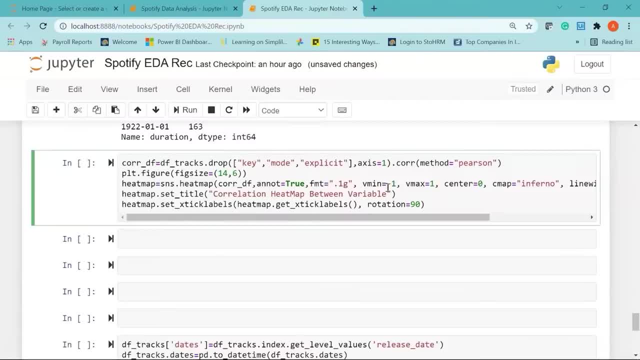 a first visualization. that is going to be a correlation map. we are going to drop three unwanted columns and those are key, mode and explicit, and then we are going to apply pearson correlation method. now i have set my figure size to 14, 6- and then we are using the seaborn heat map function to create 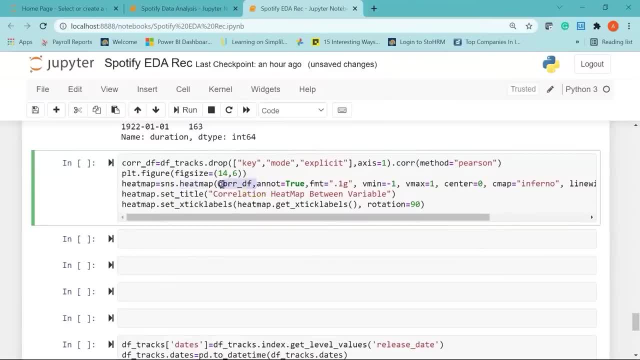 our correlation map. i have put the variable, that is correlation, underscore df. you can see above we had created this and then i'm setting annotation equal to true, so this will write the data value in each cell, set FMT equal to dot 1 G. so this is a string formatting code to use when 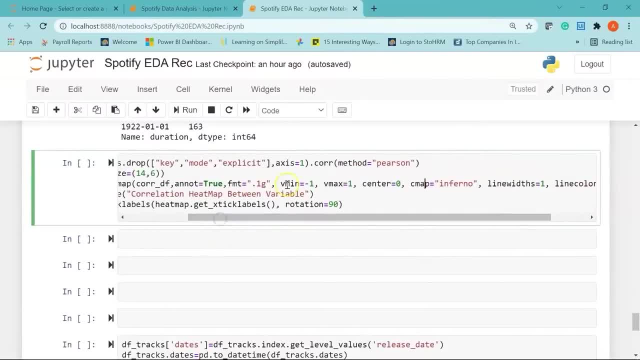 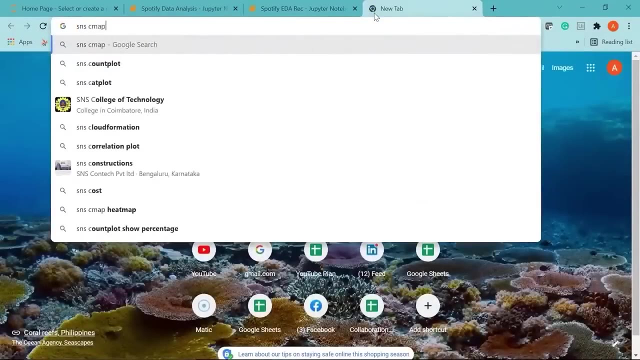 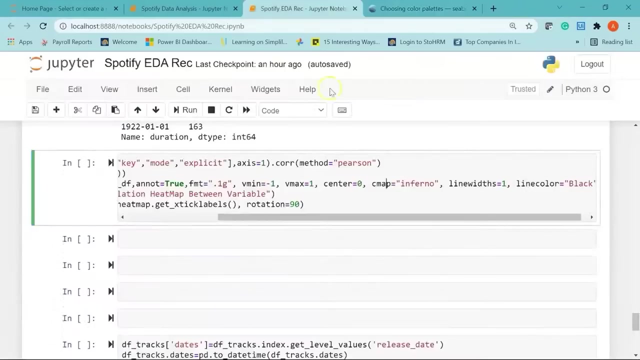 adding annotations. then I have set my V min and V max. so these are the values to anchor the color map. otherwise they are inferred from the data and other keyword arguments. CMAP here stands for color map. you can just search for SNS CMAP. you will get the documentation so you can choose whichever color palette or the. 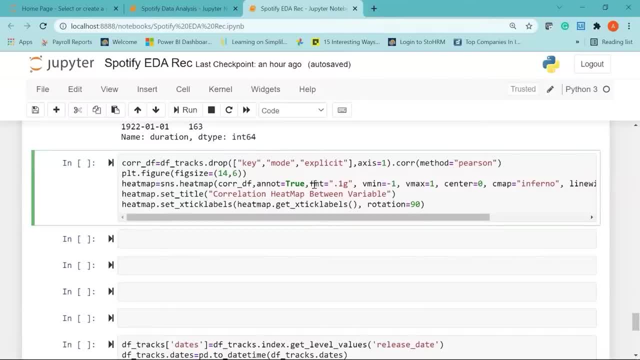 g. so this is a string formatting code to use when adding annotations. then i have set my vmin and vmax. so these are the values to anchor the color map. otherwise they are inferred from the data and other keyword arguments. cmap here stands for color map. you can just search for. 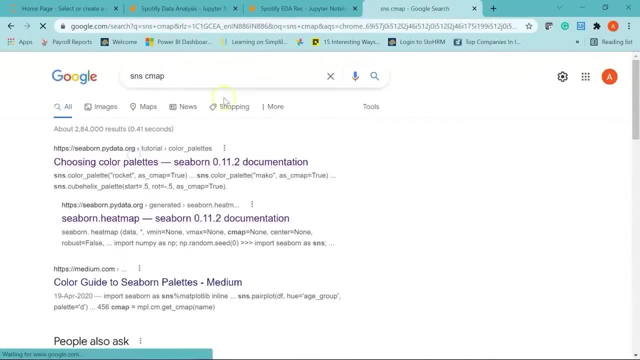 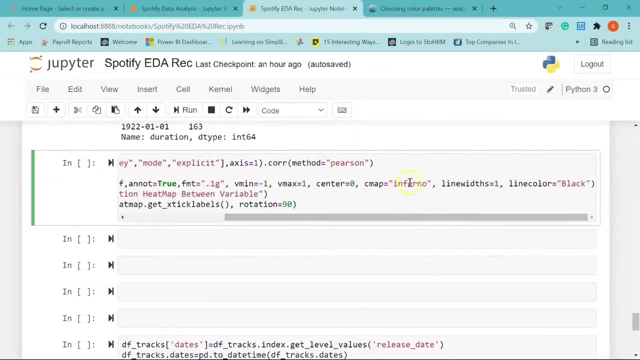 sns, cmap. you will get the documentation so you can choose whichever color palette or the color map you want. here i have used infono and i have set my line widths and line color. finally, i am giving a title to my correlation map and i have set the 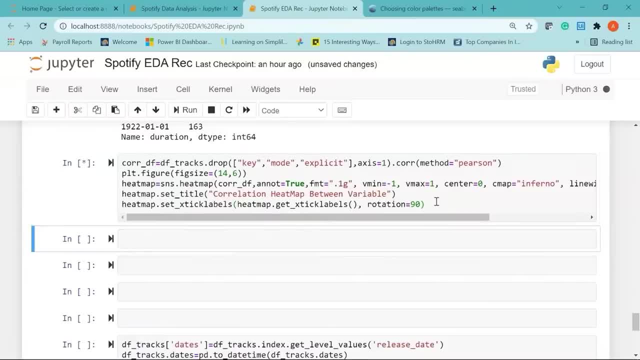 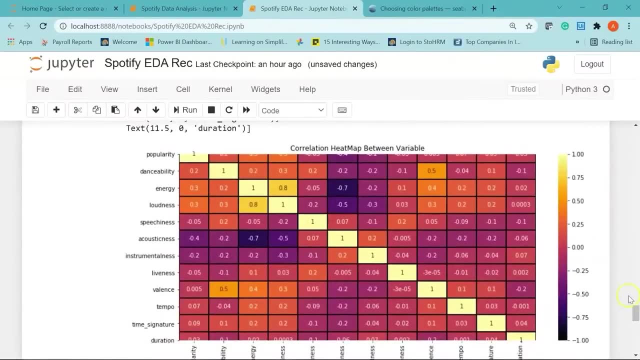 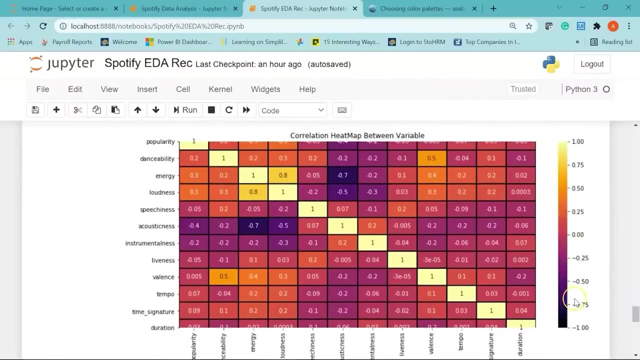 xtc labels. let's go ahead and run this to get our first visualization. if i scroll down, there you go. we have got a nice correlation map. so here on the right side you can see the scale. it ranges from minus 1 to plus 1. minus 1 means the. 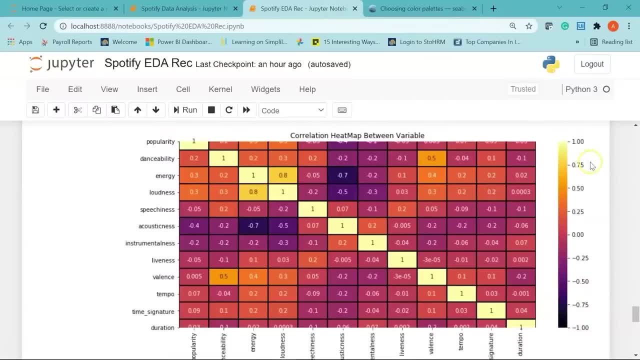 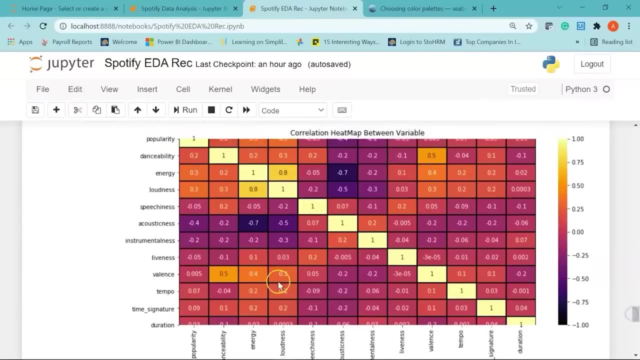 variables have least or negative correlation, while the values which are above 0.0 means that the variables have a positive correlation. now, here you can see, there are values like minus- point 7- for energy and acousticness, which means if the energy is high, the acousticness is. 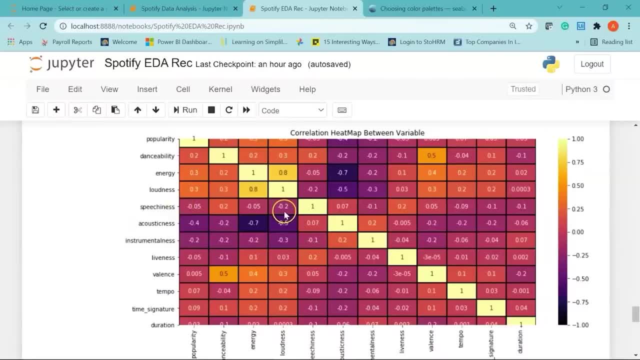 really low again for loudness and say: speechiness, if the song is loud, the speechiness is low. so there is negative correlation. but if you see for energy and loudness there is really high correlation between these two variables. you can see the value is pointed. so if the song is loud, 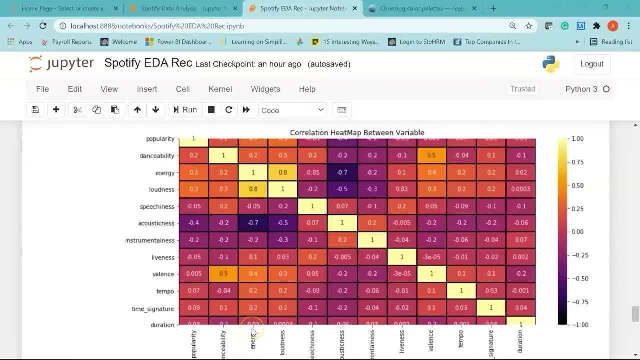 this implies the song has really high energy and vice versa. now, if you see, for a few other variables, there is negative correlation between acousticness and danceability. there is negative correlation again between valence and acousticness. similarly, there is positive correlation between energy and valence, which is 0.4. 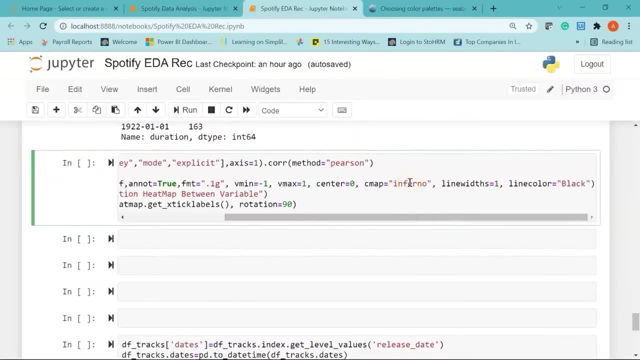 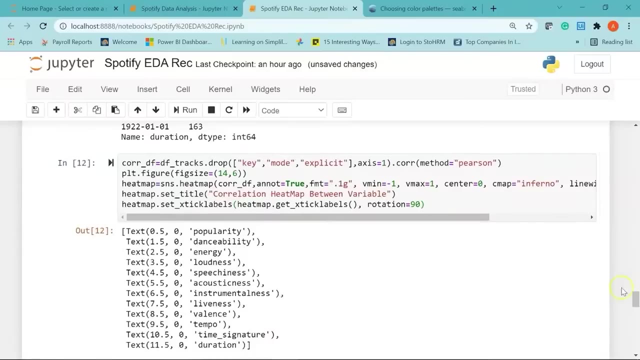 color map you want. here I have used info no, and I have set my line widths and line color. finally, I am giving a title to my correlation map and I have set the X tick labels. let's go ahead and run this to get our first visualization, if I 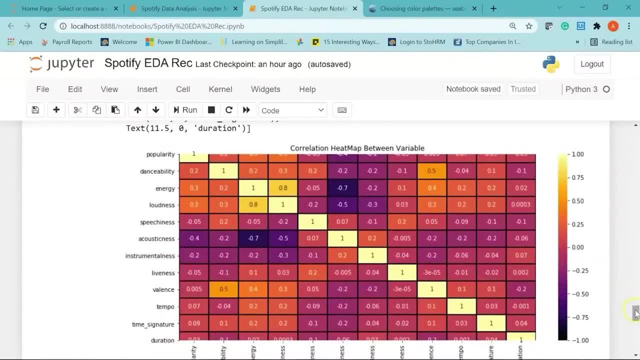 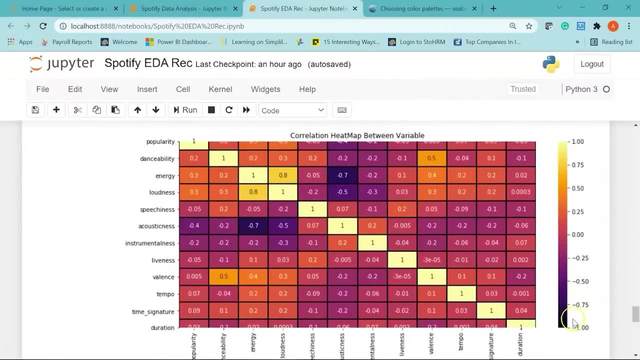 scroll down. there you go. we have got a nice correlation map. so here on the right side you can see the scale. it ranges from minus 1 to plus 1. minus 1 means the variables have least or negative correlation, while the values which are above 0.0 means that the 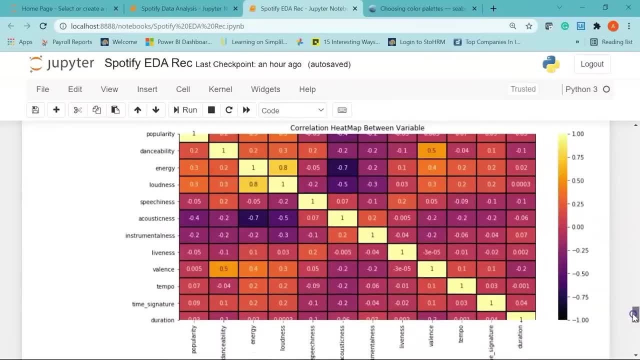 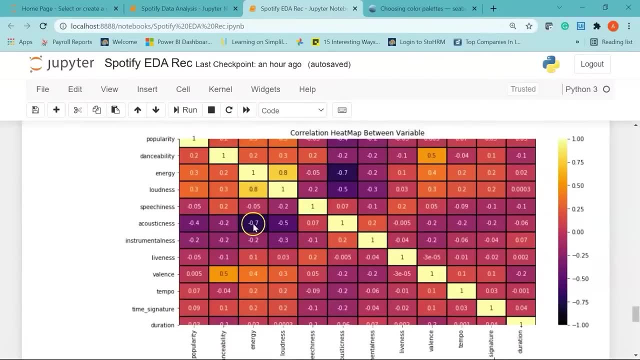 variables have a positive correlation. now here you can see there are two values like minus 0.7 for energy and acousticness, which means if the energy is high the acousticness is really low. again for loudness and say speechiness: if the song is loud the speechiness is low. so there is negative correlation. but 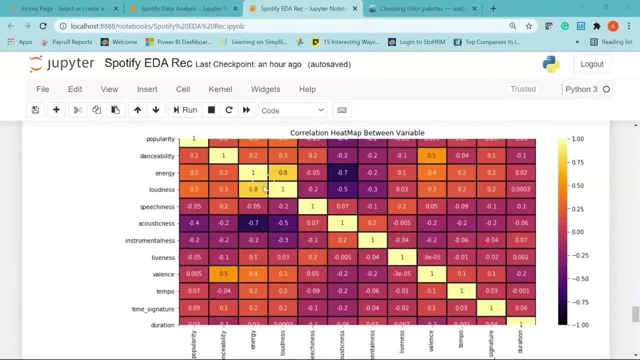 if you see for energy and loudness, there is really high correlation between these two variables. you can see the value is 0.8. so if the song is loud it is 0.4. just therefore the body can actually say voice likings. this implies 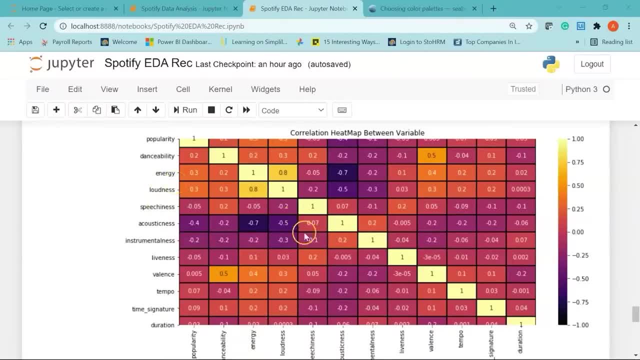 the song has really high energy and vice versa. now, if you see, for a few other variables, there is negative correlation between acoustics and dance ability. there is negative correlation again between valence and acousticness. similarly, there is positive correlation between energy and valance, which is 0.4, and even for dance ability. 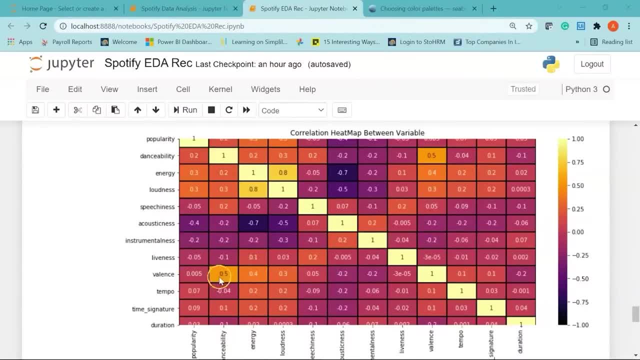 and even for danceability and valence there is positive correlation, which is 0.5. so from the correlation heatmap you can note that acousticness appears to have a strong negative correlation with energy. so if you see, for acousticness and energy there is a strong 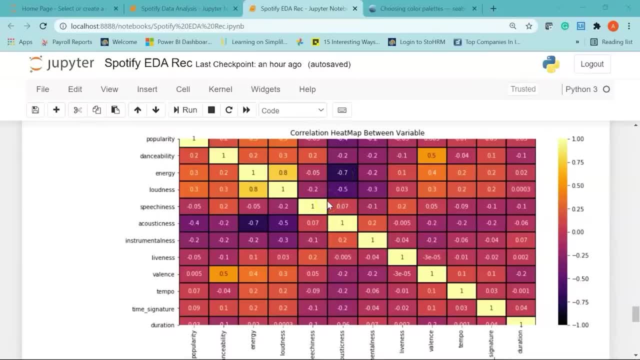 negative correlation and there is a moderately strong positive relation between loudness and popularity. so if you see, for popularity and loudness the color is orange, which means it lies in this positive region, and there is also a moderately strong positive relation between danceability and valence. 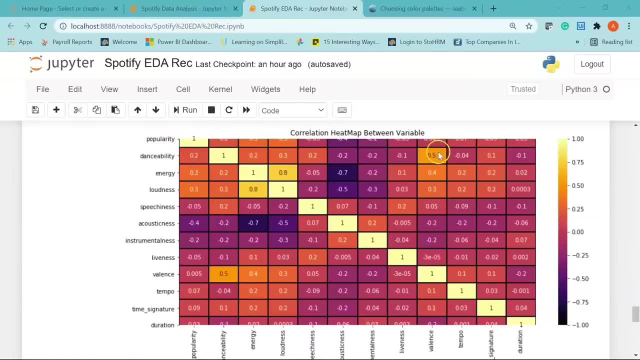 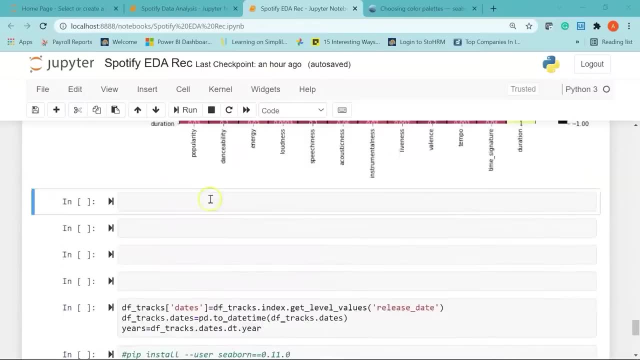 so if you check for danceability and valence here, there is a moderately strong positive correlation. alright, now let's move ahead. we are going to sample our data and take just 0.4% of the total data, and we will create two regression plots using this data. 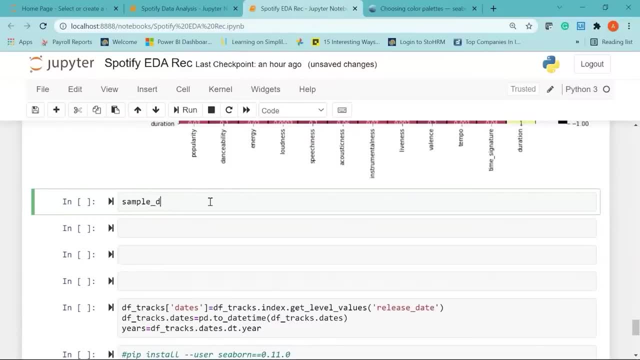 so let me first sample my data. so i will create a sample data frame using my original data frame, which is df, underscore tracks, and say sample. i am going to use the int function and say 0.004 multiplied by the length of my original data frame, which is: 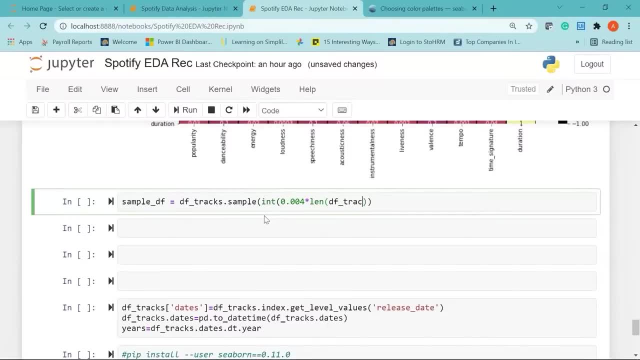 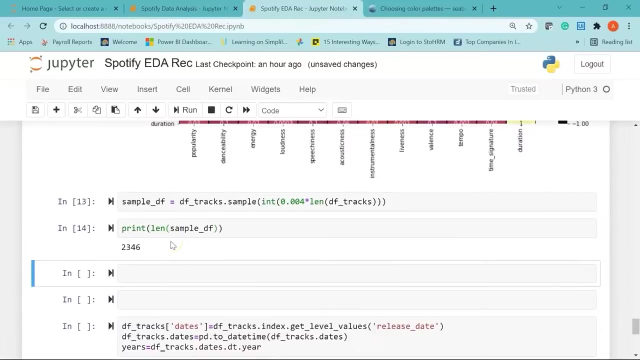 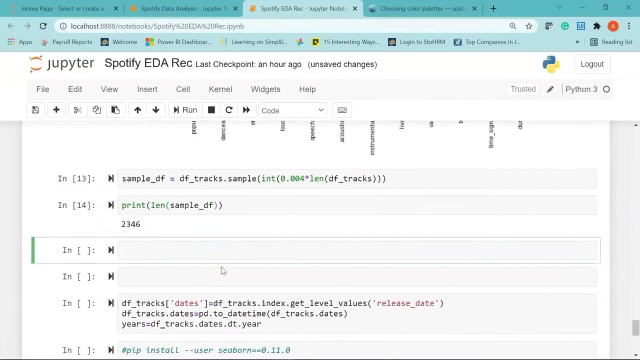 df underscore tracks. alright, now let's run this and we will print the length of my sample data frame. if i run it, you can see 0.4% of my total data set is 2346 rows. cool, now we are going to create a regression plot between: 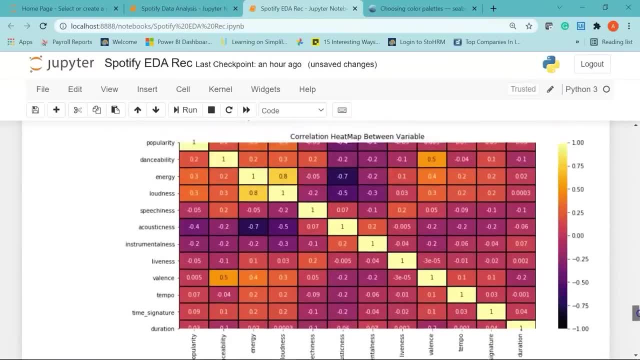 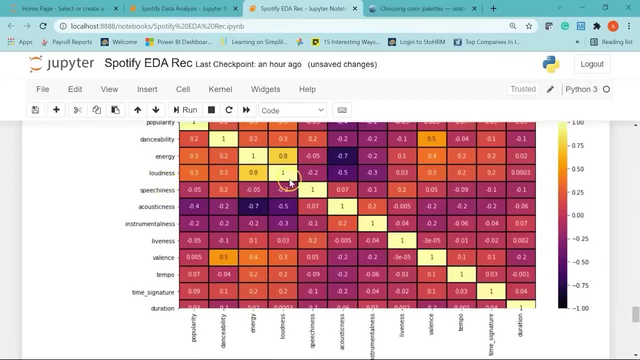 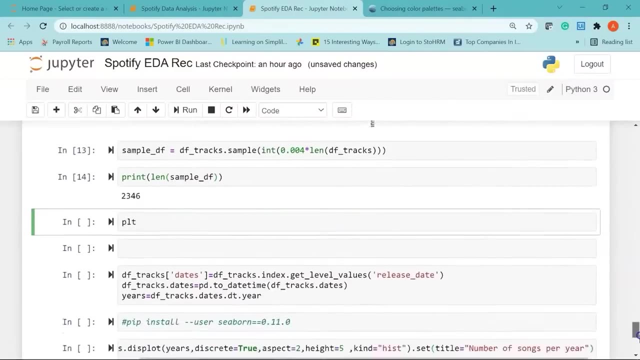 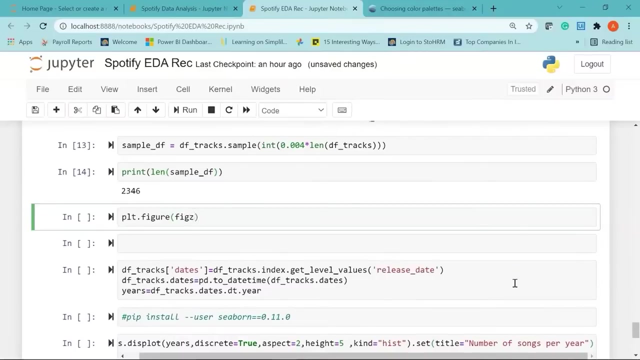 loudness and energy. now in our correlation map we saw there was a positive correlation between loudness and energy which was 0.8. let's plot it in the form of a regression line. so i will use plt dot figure. i will set my number size. 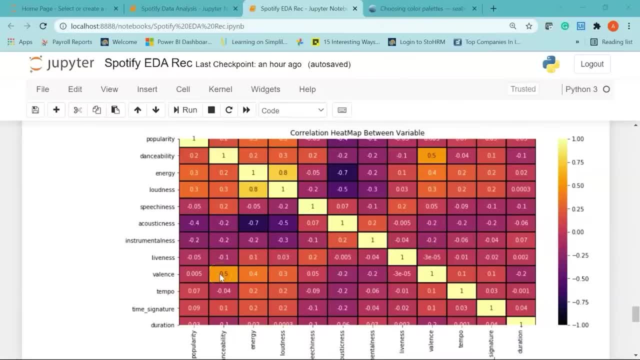 extensibility and valence. that is positive correlation which is 0.5 cool. So from the correlation heat map you can note that acousticness appears to have a strong negative correlation with energy. So if you see, for acousticness and energy there is a strong negative correlation and there 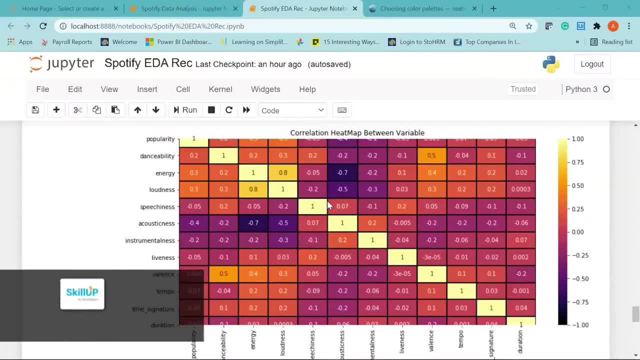 is a moderately strong positive relation between loudness and popularity. So if you see, for popularity and loudness the color is orange, which means it lies in this positive region, and there is also a moderately strong positive relation between densibility and valence. So if 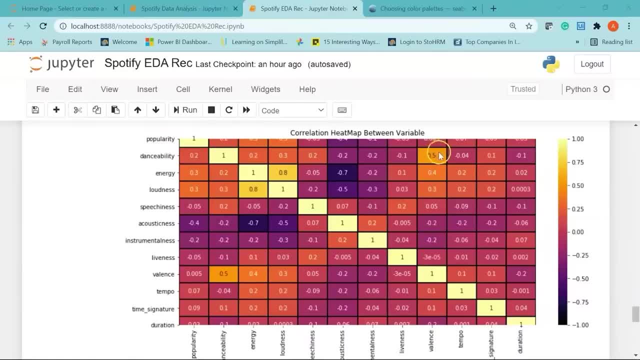 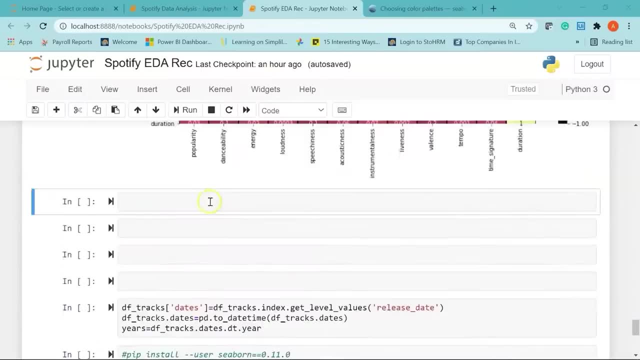 you check for densibility and valence, here there is a moderately strong positive correlation. All right, now let's move ahead. We are going to sample our data and take just 0.4 percent of the total data and take a look at the correlation heat map. So if you see for acousticness and 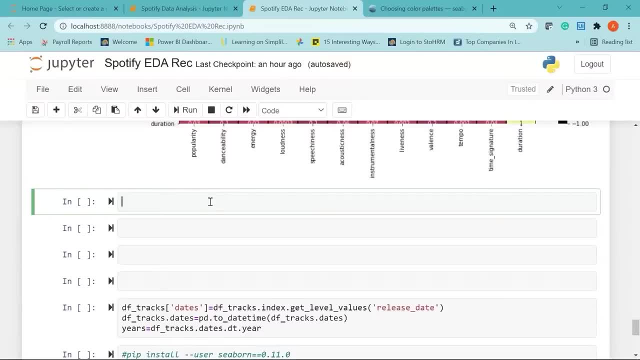 I will create two regression plots using this data. So let me first sample my data. so I will create a sample data frame using my original data frame, which is DF, underscore tracks and say sample. I'm going to use the int function and see 0 point 0, 0, 4 multiplied. 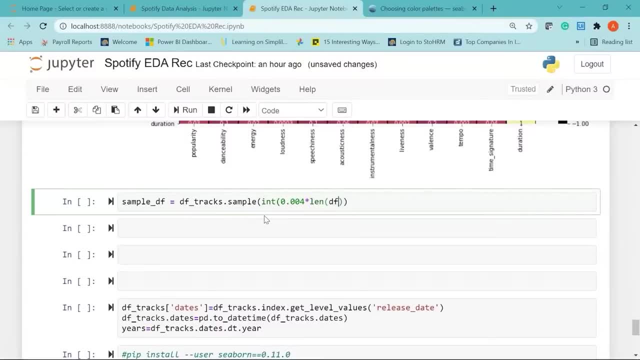 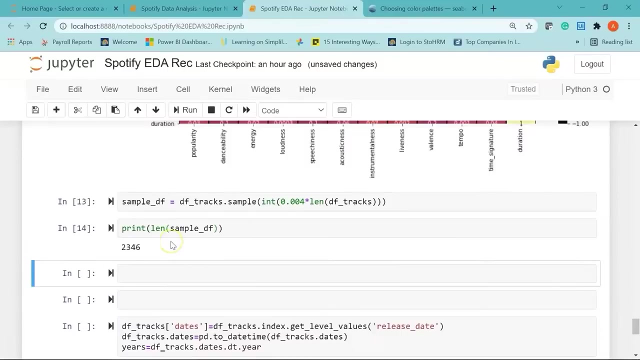 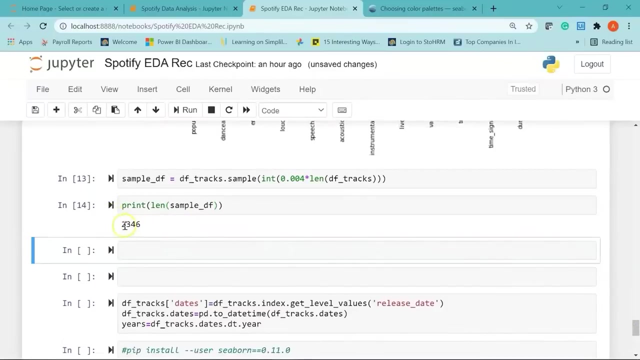 by the length of my original data frame, which is DF underscore tracks. all right, now let's run this and we'll print the length of my sample data frame. run it, you can see. point four percent of my total data set is two thousand three hundred and forty six rows. cool, now we are going to create a regression plot between: 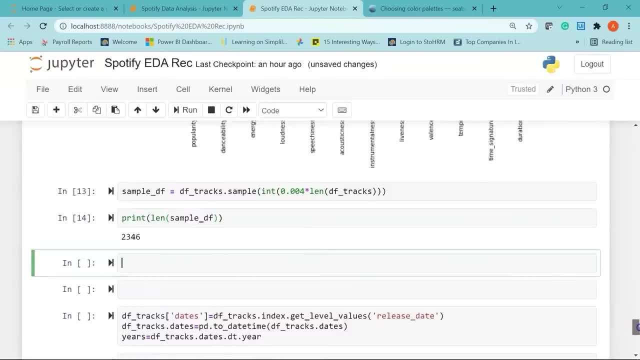 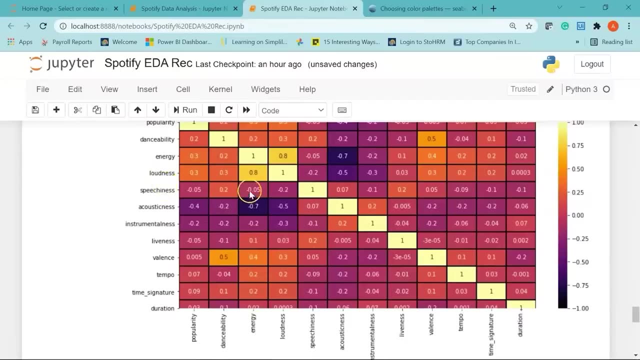 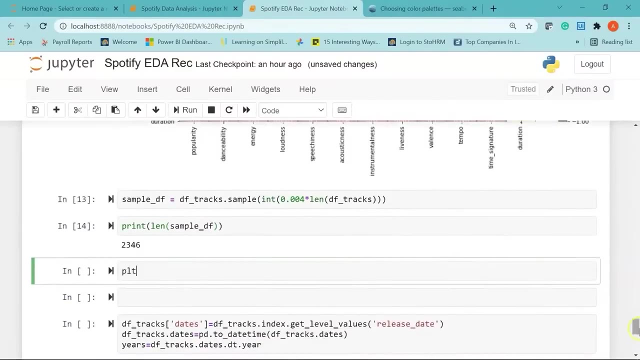 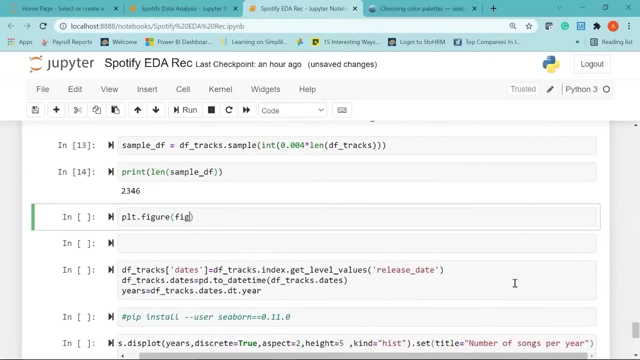 loudness and energy. now in our correlation map we saw there was a positive correlation between loudness and energy which was pointed. let's plot it in the form of a regression line. so I'll use PLT dot figure. I'll set my figure size equal to, let's say, 10 comma 6. I will say: 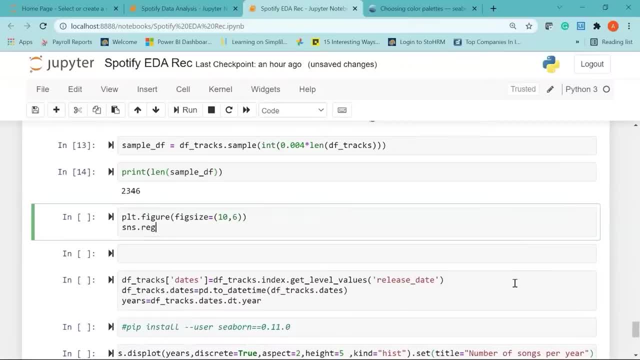 SNS dot regression plot. so I'm using SNS dot regression plot. so I'm using SNS dot regression plot. so I'm using the function called reg plot and I'll use my data as sample underscore EF. give a comma and say: in my y-axis I'll have my column loudness and in the x-axis we'll have energy, I'll give a color to. 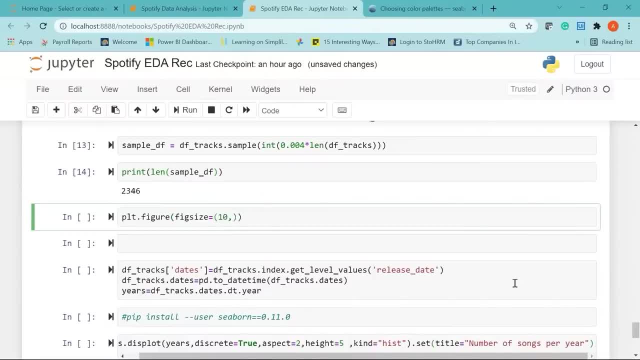 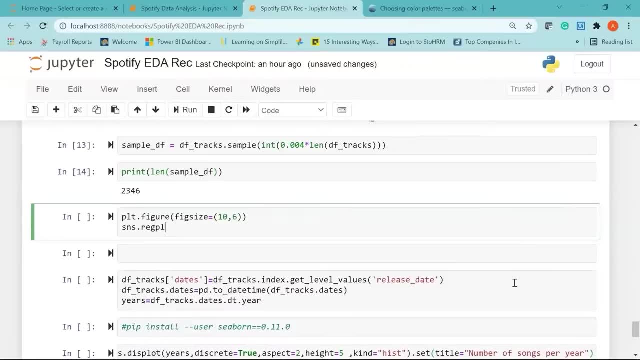 equal to, let's say, 10 comma 6, i will say sns dot regression plot. so i am using the function called regplot and i will use my data as sample. underscore df, give a comma and say: in my y axis i will have my column loudness. 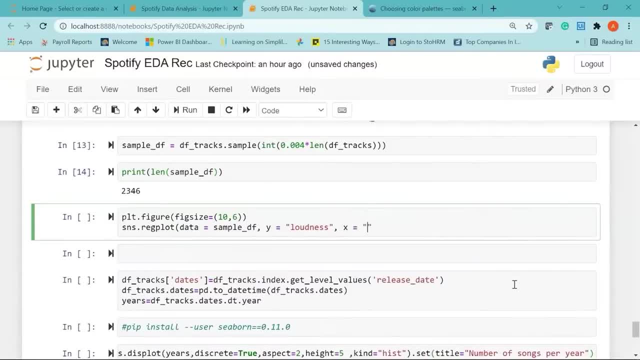 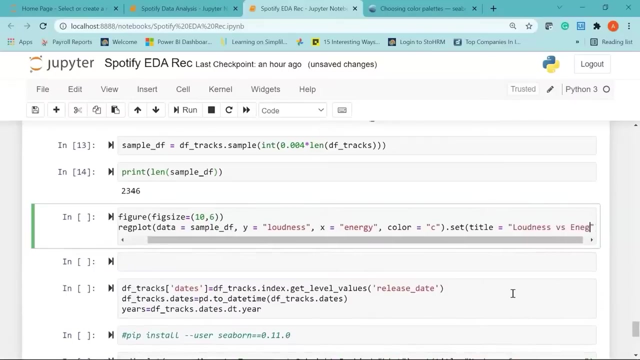 and in the x axis we will have energy. i will give a color to my data variable. let's say the color is c. then i will set my title to loudness versus energy. let's say correlation. alright, let's make sure everything is fine. now we will run. 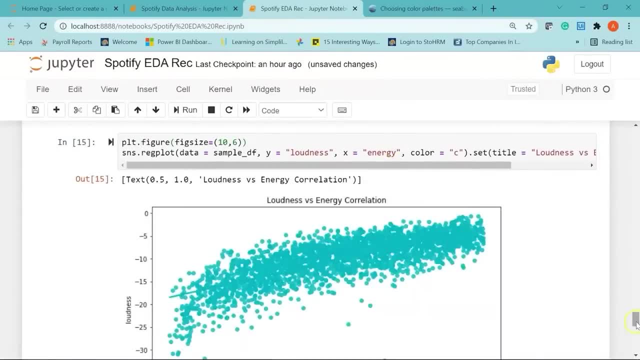 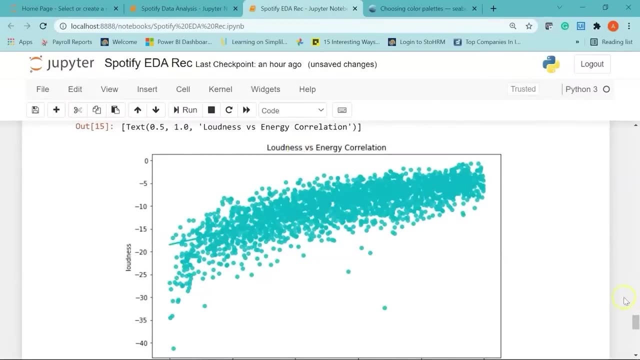 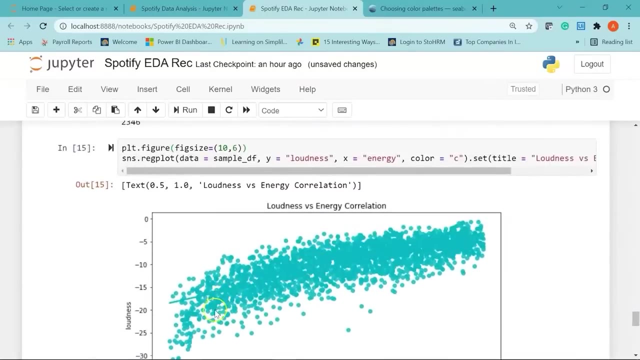 and see our result. there you go, so you can see here clearly there is a very high positive correlation between loudness and energy. on the y axis we have loudness and on the x axis we have energy, and you can see all the data points or the songs are: 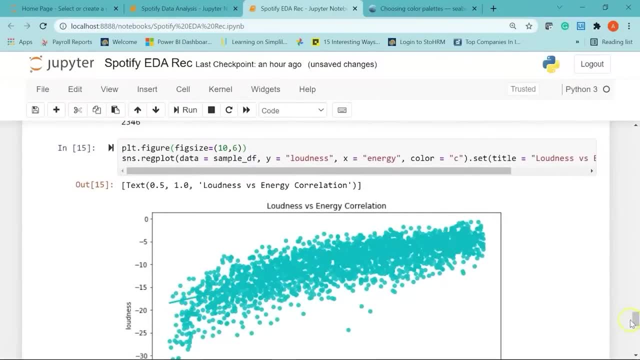 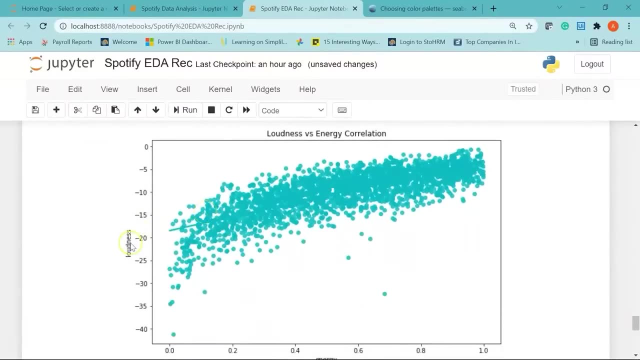 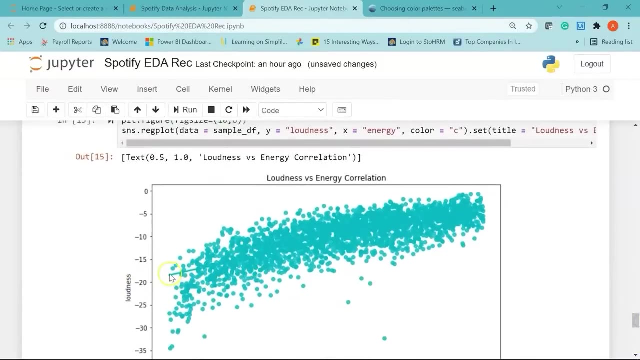 in one direction. so if the energy increases, the loudness of the song also increases and similarly, if the loudness of the song decreases, your energy of the song or the track also decreases. so there is a very high positive correlation and you can see the regression line here. it has gone. 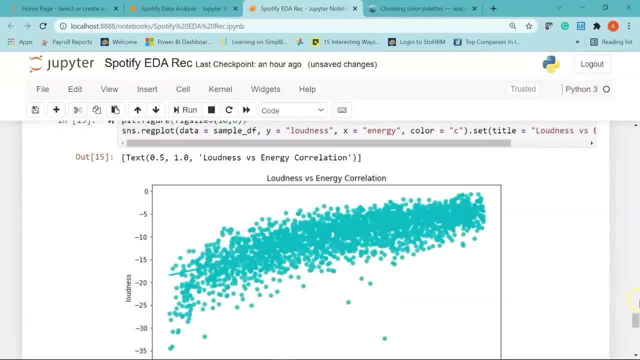 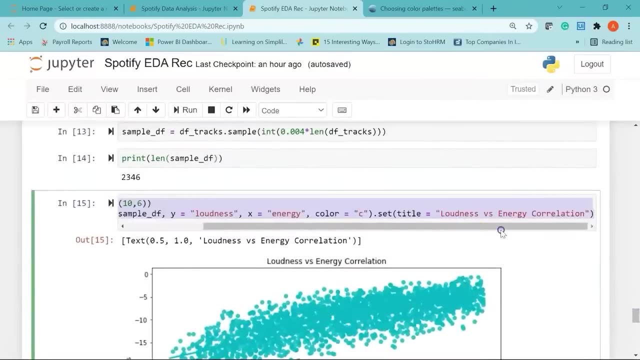 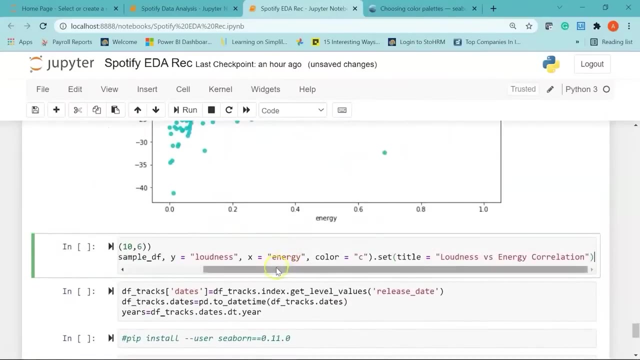 and is increasing gradually. cool now. similarly, i will just copy this code and we are going to see another regression plot, this time for two different features. let's say we have popularity in the y axis, so i will say popularity. and then in the x axis we have, let's say, 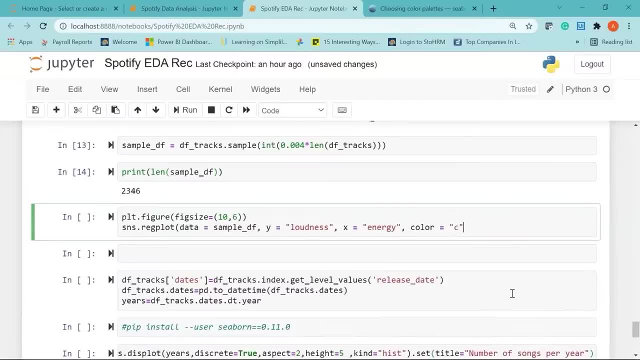 my column loudness, and in thexy axis we'll have energy and in the y-axis we'll have energy. my column loudness, and in thexy axis we'll have energy and in the x-axis we'll have energy. my data variable, let's say the color, is C, then I will set my title to: 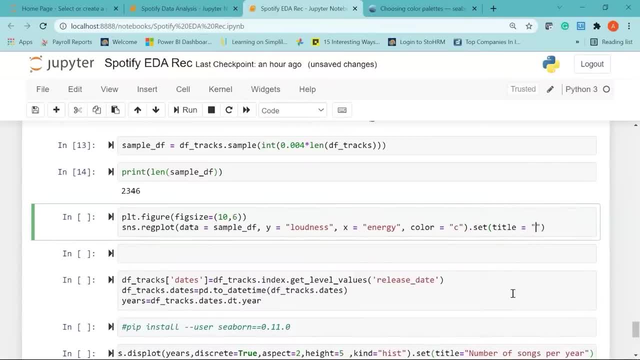 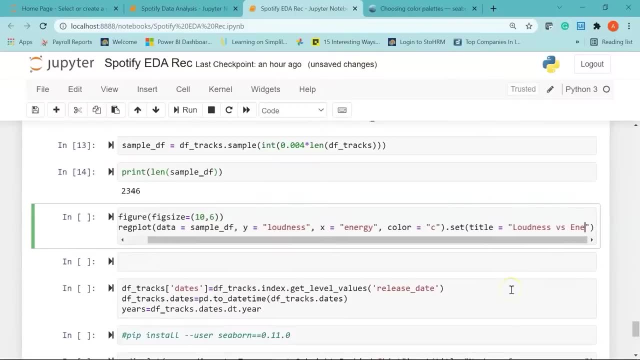 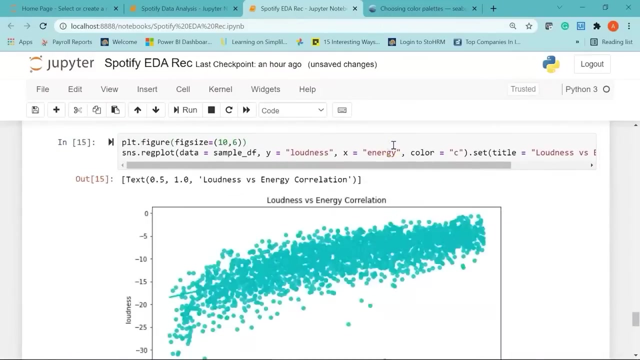 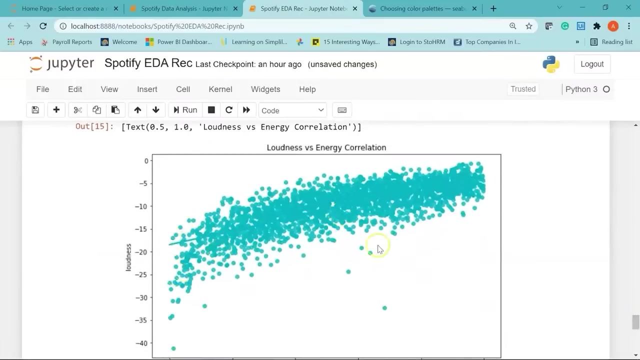 loudness, Bo privileges. let's say correlation again. let's say correlation again. alright, all right. good, let's make sure everything is fine. now we'll run and see a result. there you go. so you can see here clearly there is a very high positive correlation between loudness and energy. on the 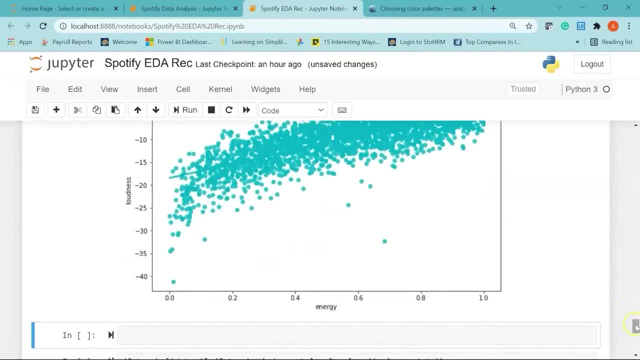 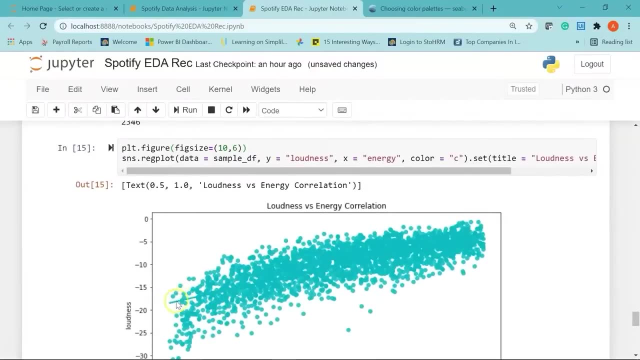 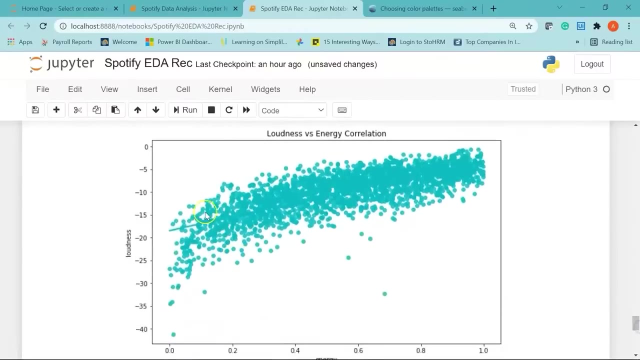 y-axis we have loudness and on the x-axis we have energy, and you can see all the data points for these songs are in one direction. so if the energy increases, the loudness of the song also increases and similarly, if the loudness of the song decreases, your energy of the song or the 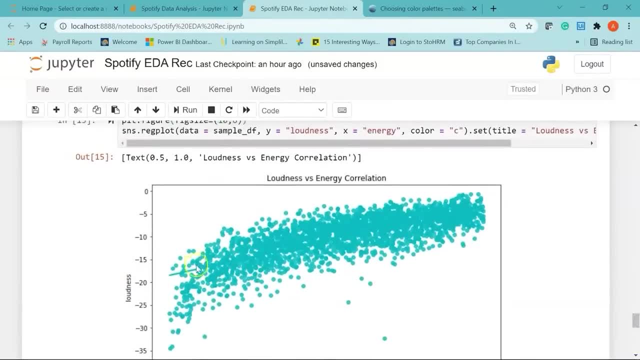 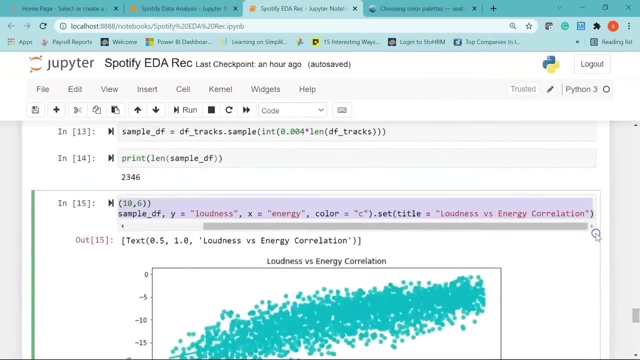 track also decreases. so there is a very high positive correlation and you can see the regression line here has gone and is increasing gradually. who now? similarly? I'll just copy this code and we are going to see another regression plot, this time for two different features. let's say we have 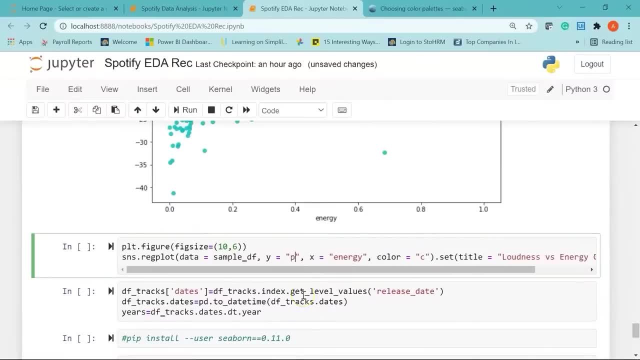 popularity in the Y axis. so I'll say popularity and then x-axis. we have, let's say, a, cost thickness. I'll change the color to, let's say, B, which stands for blue, and will set the title to popularity versus. I'll have the cost thickness correlation, the scroll down and we'll run it to see the result. 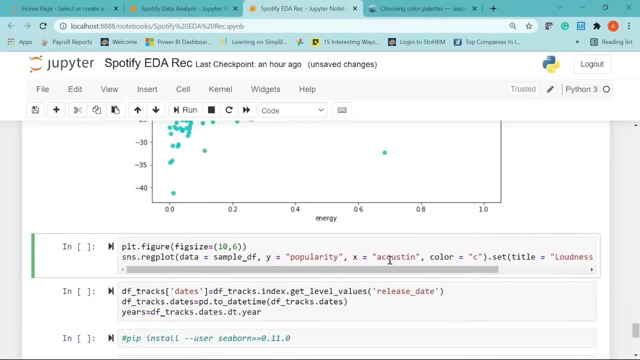 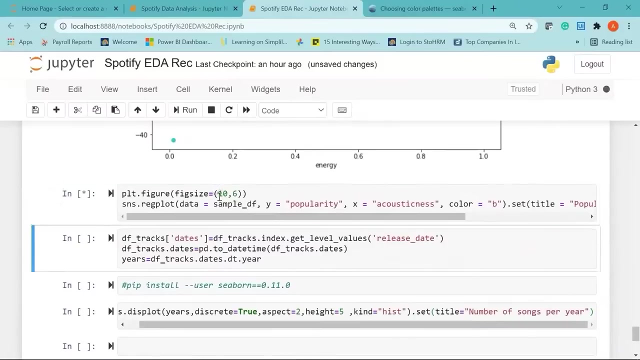 acousticness, i will change the color to, let's say, b, which stands for blue, and we will set the title to popularity versus the. i will have acousticness correlation. just scroll down and we will run it to see the result. there you go. so i have the. 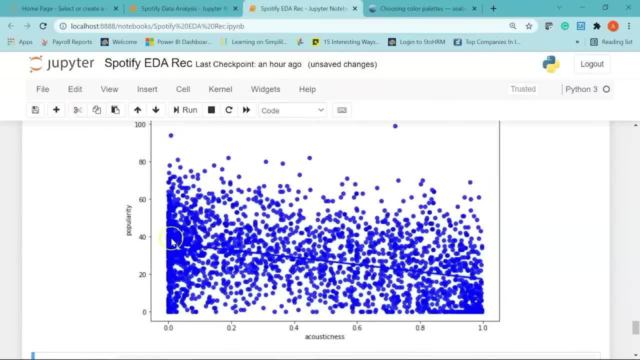 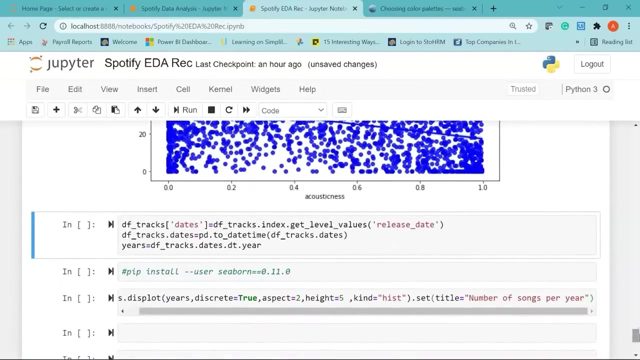 different points for the songs, and here you can see the regression line is down, which means if the acousticness of the song increases, the popularity decreases, and similarly, if the popularity increases, the acousticness decreases. you can see the downward trend of the regression line. alright, now in the next cell we are: 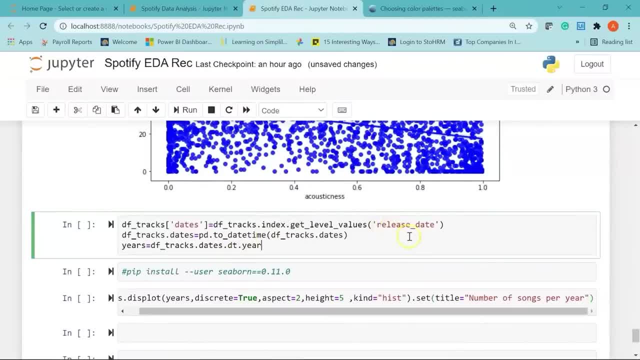 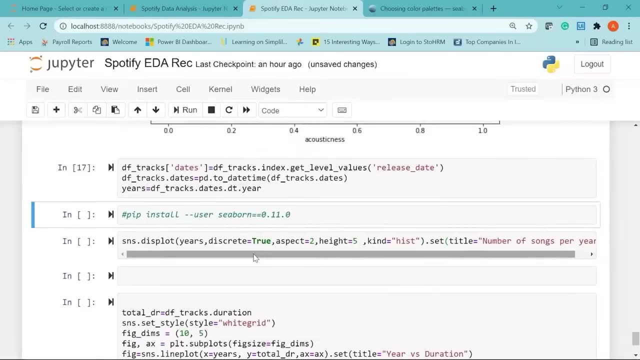 going to create a new column called year from our release date column, and i have changed this to date time format. let me just run it cool now. after that we are going to create a distribution plot to visualize the total number of songs in each year since 1922. 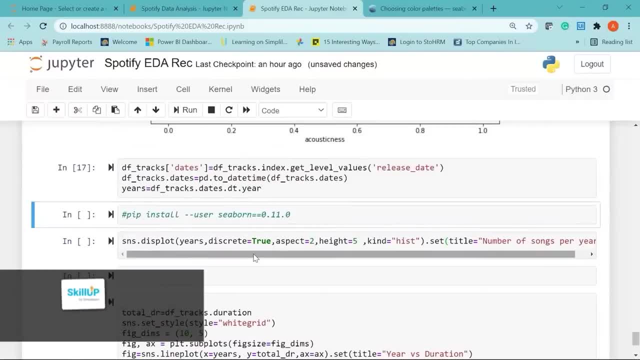 that is available on the spotify streaming app. so i have used my seaborn library and dist plot function. now, one thing to remember: you need to update your seaborn library to this version. if you haven't done it, so use this command: pip install dash dash. user seaborn and. 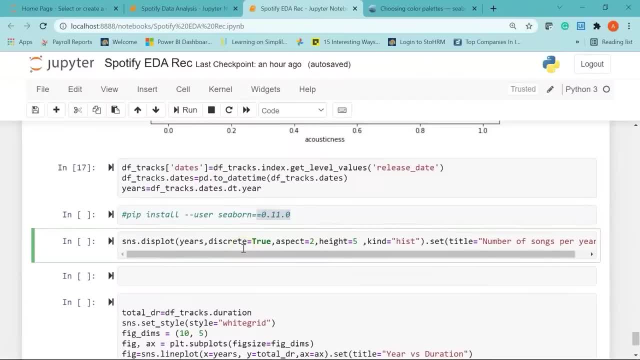 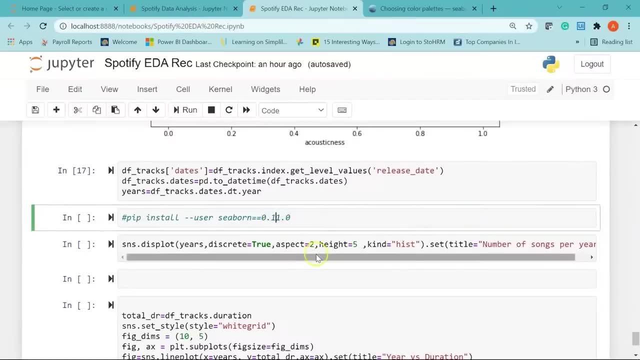 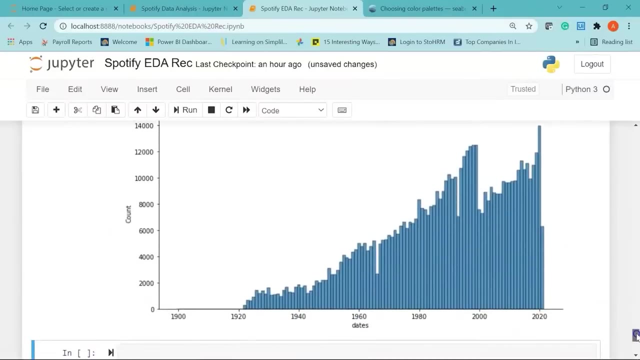 the version. so here in the distribution plot we are going to plot a histogram, so i have used kind equal to hist, which stands for histogram. let's run and see the result. ok, so here you can see, i have my distribution plot. so the plot tells us that the 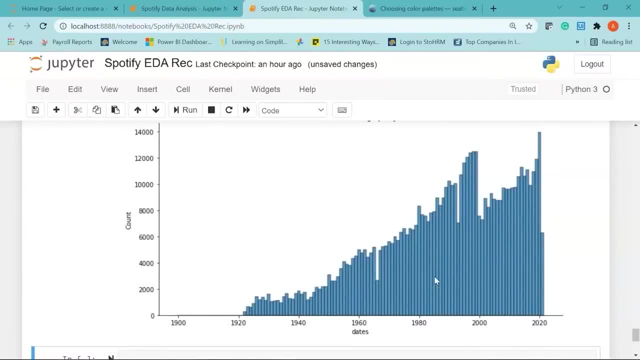 number of songs for each year in the data set according to their release date have increased in the recent years since music became more accessible to people globally with technological advancements. so earlier you can see, there were very few songs available in the 1920s. later on the 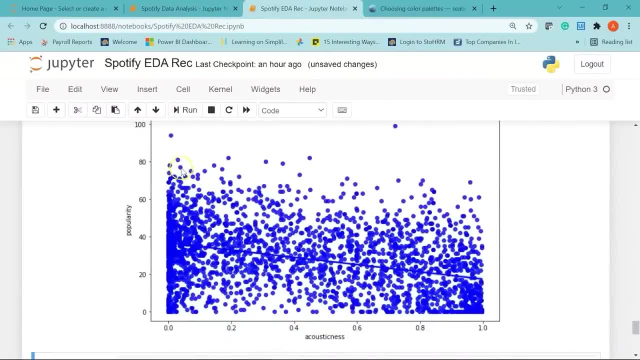 there you go. so I have the different points for the songs and here you can see the regression line is downwards, which means if the cost thickness of the song increases, the popularity decreases and similarly, if the popularity increases, the cost thickness decreases. you can see the downward trend of the regression line all right now in the 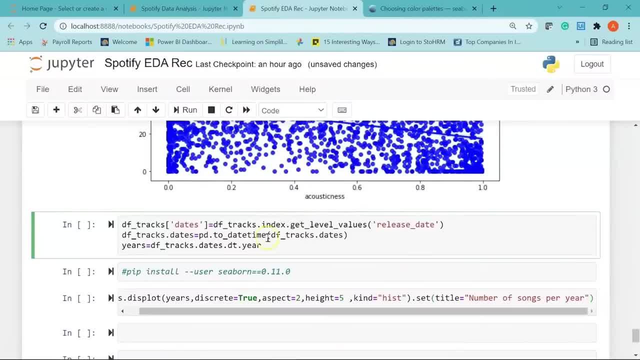 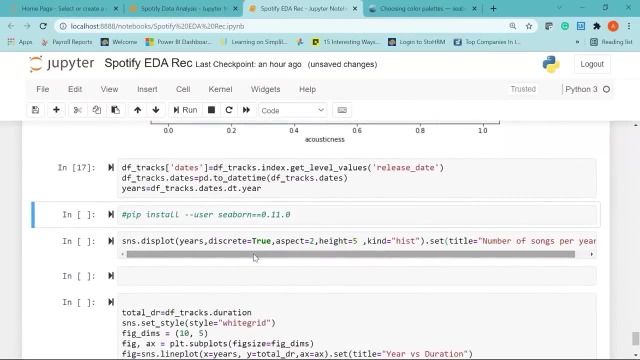 next cell, we are going to create a new column called year from our release date column and I have changed this to date time format. let me just run it cool now. after that, we are going to create a distribution plot to visualize the total number of songs that we are going to create and we are going to create a distribution plot to visualize the total number of songs. 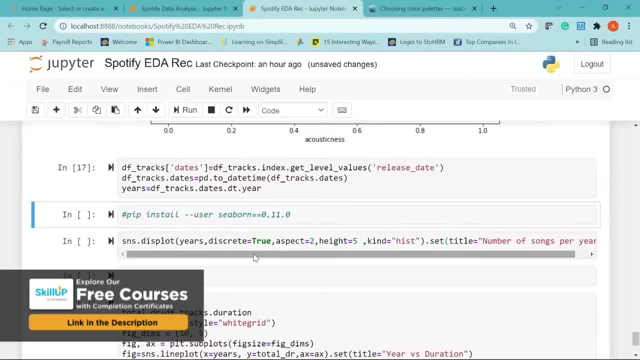 that is available on the Spotify streaming app. so I have used my seabourn library and dist plot function. now, one thing to remember: you need to update your seabourn library to this version. if you haven't done it, so use this command: pip install dash, dash, user, seaborn and the version. so here in the distribution plot you. 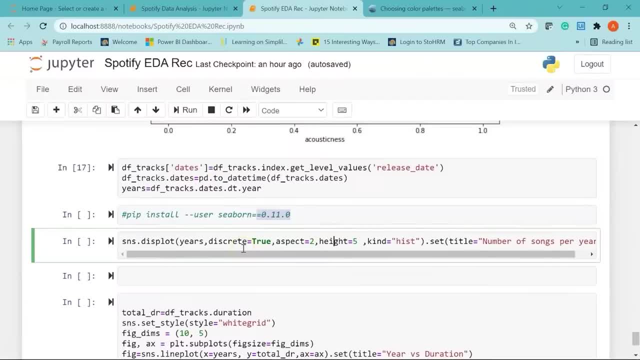 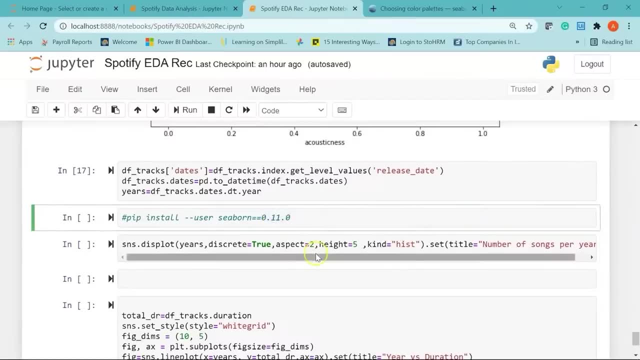 cannot click on that here. you just have to click on that and you are left with this seabourn order and you are now running right on top. Ok, so thatї. Here in the distribution plot we're going to plot a histogram, So I've used kind equal to hist, which stands for histogram. 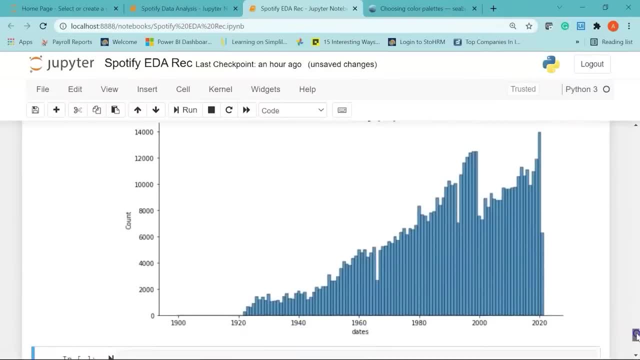 Let's run and see the result. OK, so here you can see. I have my distribution plot. So the plot tells us that the number of songs for each year in the data set according to their release date, have increased in the recent years, since music became more accessible to people globally. 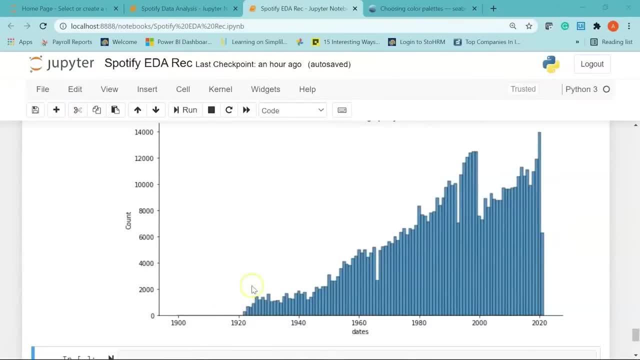 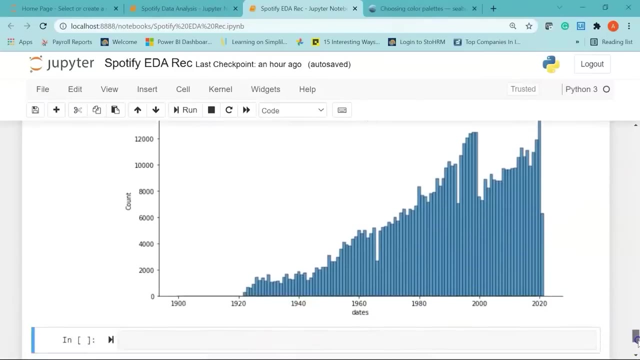 with technological advancements. So earlier you can see, there were very few songs available in the 1920s. Later on the number of songs increased rapidly And now you can see we have a lot more songs available for people to listen. Cool. 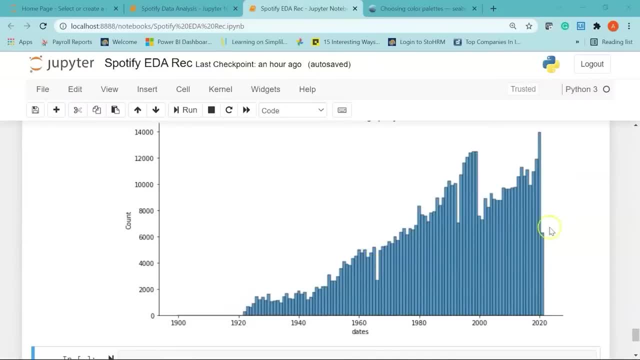 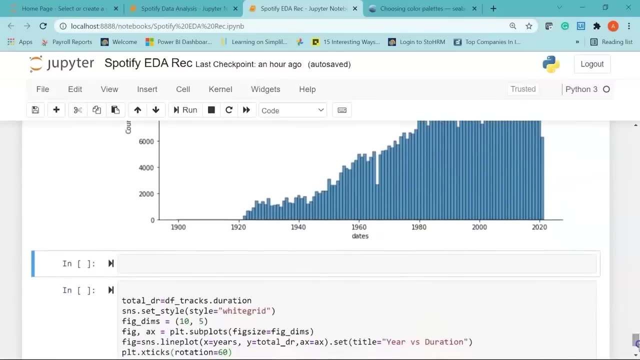 number of songs increased rapidly and now you can see we have a lot more songs available for people to listen. cool, now we are going to see the duration of songs over the years. for that again, we are going to create a bar plot. so i will first create a. 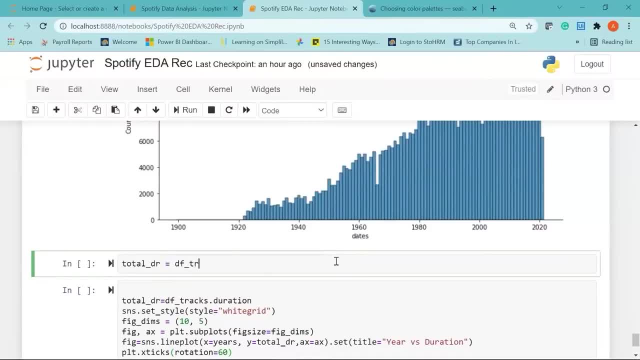 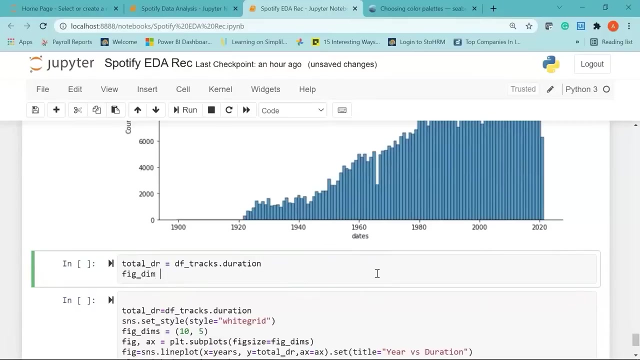 variable called total duration equal to df underscore tracks dot. i will use the duration column that we created with seconds, and then i am going to set my figure dimensions. so i will use figure underscore dims for dimensions equal to 18 comma 7. after that i will have my 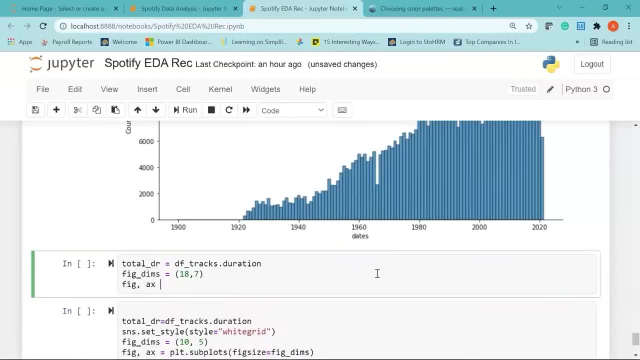 figure axis defined. so i will use the matplotlib subplots function and i will set the figure size equal to my figure dimensions and then i will say figure equal to sns dot. i will use the barplot function and say my x-axis to be years. my y-axis will be: 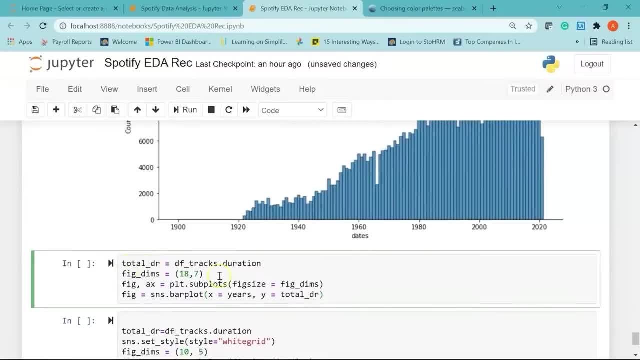 total duration or total underscore dr that we created here. i will set my axis equal to ax and then i will set error width equal to false. let's set the title for my plot as title equal to year bosses duration and finally i will say plt dot. i will rotate it by. 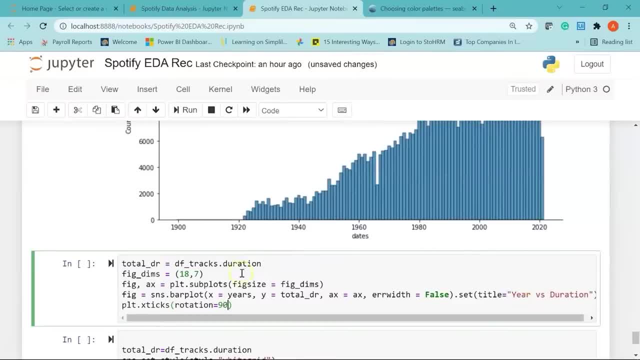 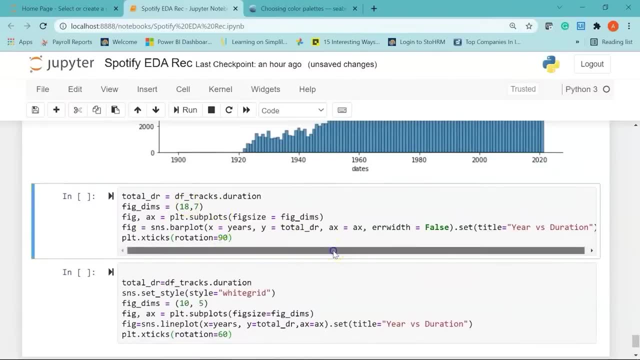 let's say 90 degrees. all right, let me just recheck once if everything is fine, and then we will go ahead and run it. i have my axis error width title. ok, let me just run it. we will see the result in a moment if i scroll down, you can. 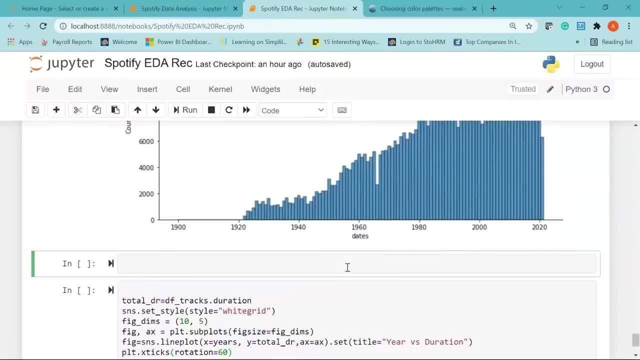 Now we are going to see the duration of songs. So we are going to see the duration of songs over the years. For that again we are going to create a bar plot. So I'll first create a variable called total duration, equal to df. underscore tracks, dot. 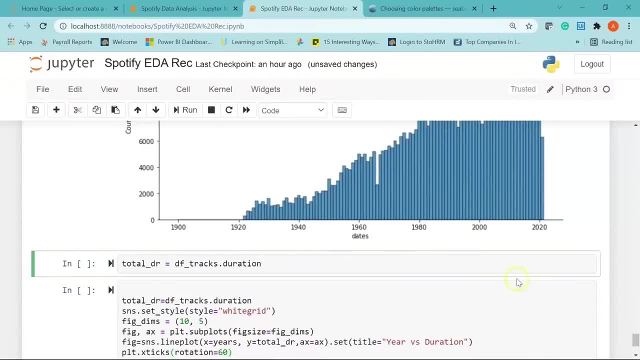 I'll use the duration column that we created with seconds, And then I'm going to set my figure dimensions. OK, So I'll use figure underscore dims for dimensions equal to 18,7.. After that, I'll have my figure axis defined. 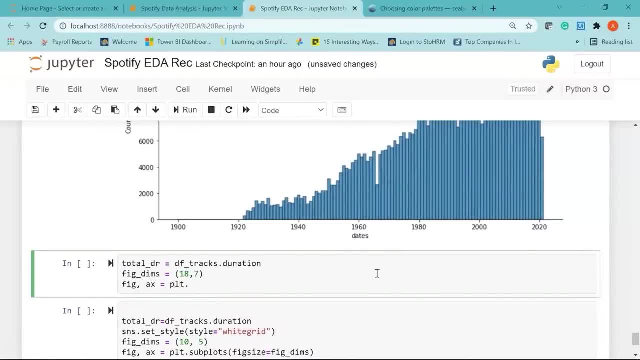 So I'll use the matplotlib subplots function And I'll set the figure size. So I'll use my figure size equal to my figure dimensions And then I'll say figure equal to sns dot. I'll use the barplot function And say my x-axis to be years. 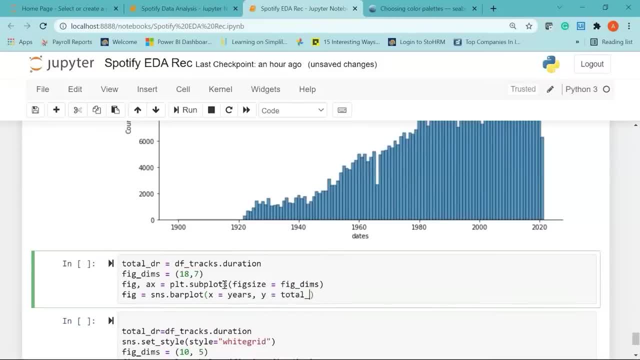 My y-axis will be total duration or total underscore dr that we created here. I'll set my axis equal to ax and then I'll set error width equal to false. Let's set the title for my plot as title equal to year bosses duration and finally I'll say: 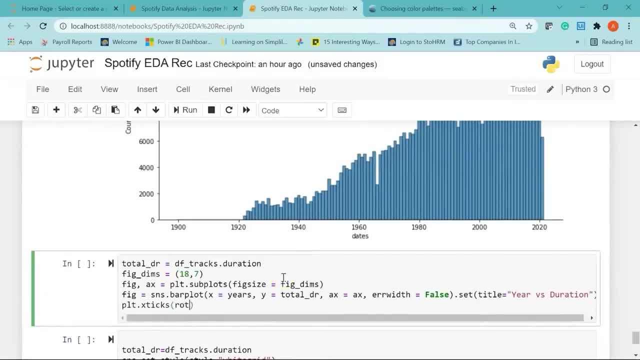 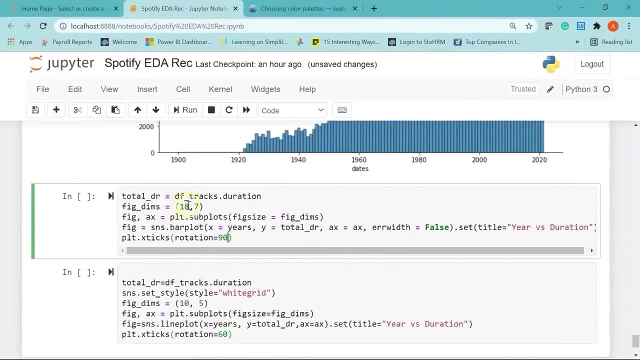 pltxtex. I'll rotate it by, let's say, 90 degrees. All right, let me just recheck once if everything is fine, and then we'll go ahead and run it. I have my axis error width title. Okay, let me just run it. 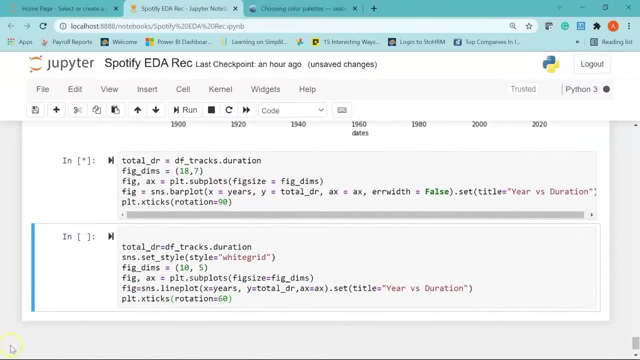 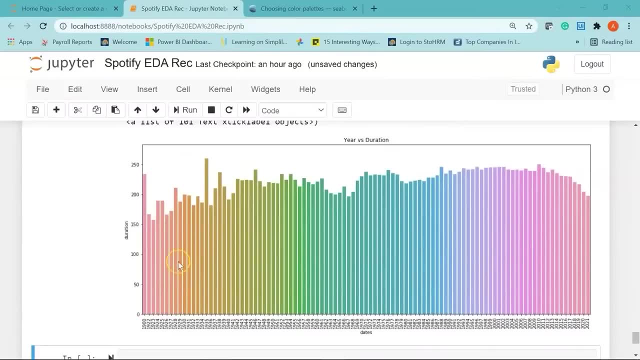 We'll see the result in a moment. If I scroll down you can see we have the bar plot for the different years and the duration of the songs in seconds in the y-axis. So earlier in the 1920s you can see the duration of the songs were less and later it increased. 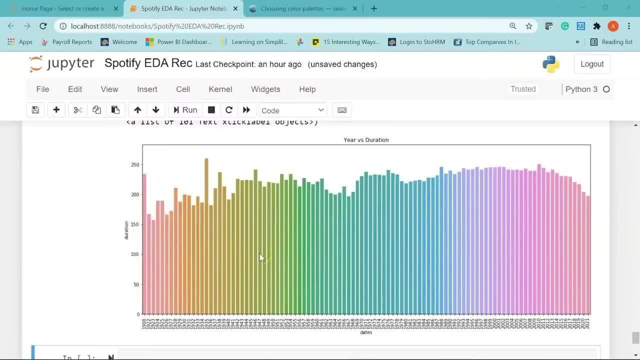 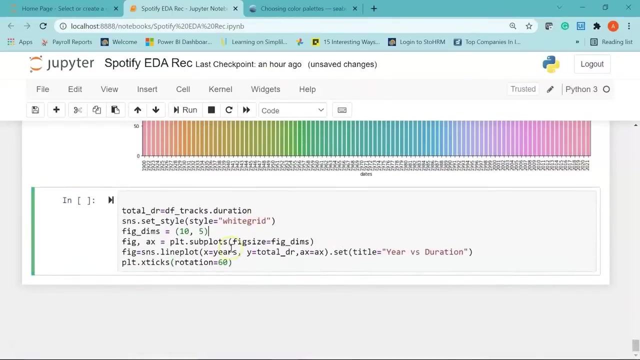 around late 1930s and this remained consistent until 2010, where the duration was high. But after 2010, you can see the duration of the songs have started decreasing. Now, in the next year, Next cell, I'm going to create a line plot to analyze the average duration of the songs. 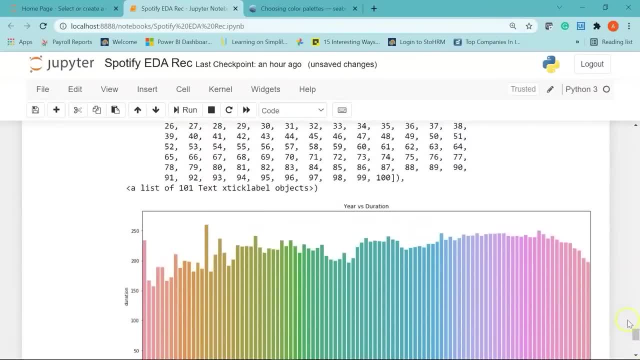 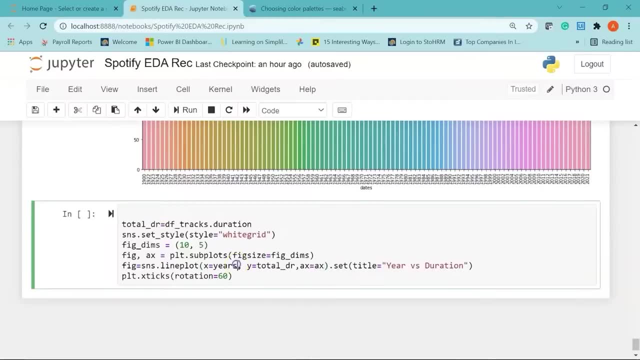 over the years. It is going to be similar to a bar plot, Just that. now we are going to visualize it in terms of a line. So I have my code ready. You can see here I've used my seaborn library and the line plot function in the x-axis. 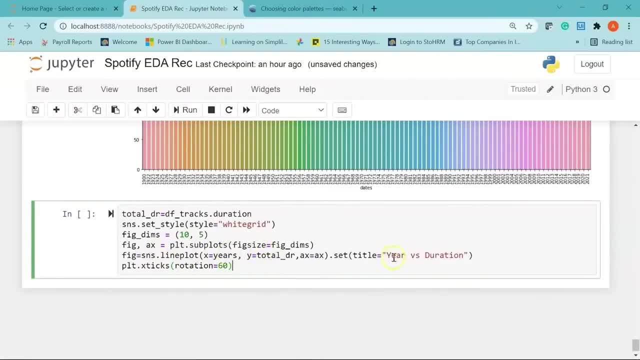 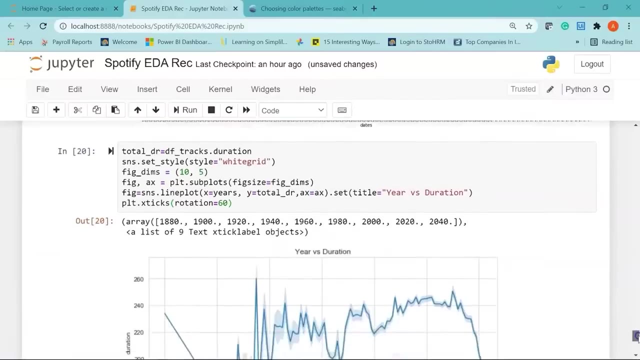 I have years and in the y-axis I have total duration. I've set my title to year bosses duration- year versus duration, and I am rotating my x labels by 60 degrees. Let's run it and we will see the output. There you go Now. if I scroll down, you can see: 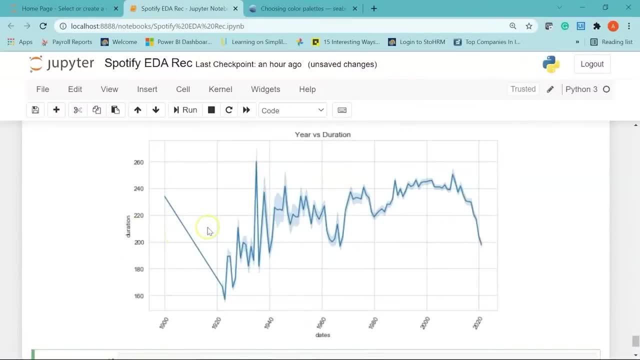 we have a nice line plot, and on the x axis you have the years and on the y axis we have the duration. You can see that the songs from 1920s to 1960s have comparatively shorter duration, since most of the songs tended to be more singing based rather than 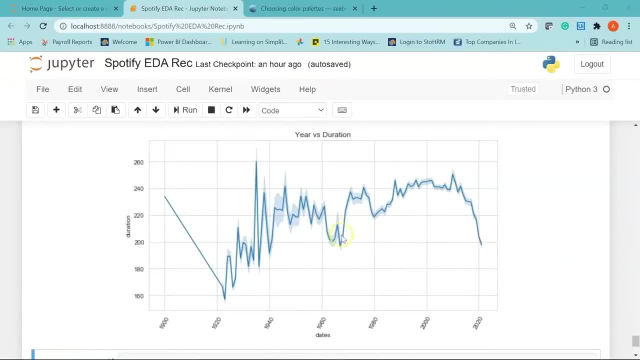 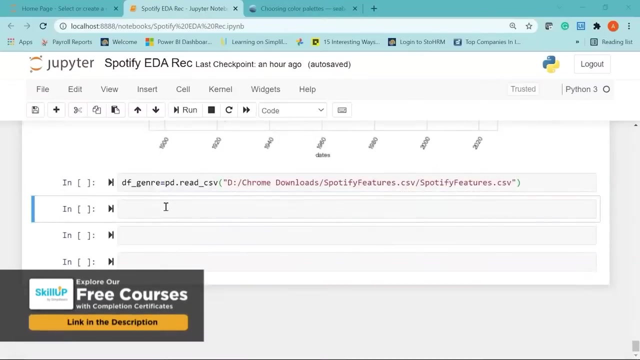 instrument based After 1960s, you can see the duration of the songs started increasing until, I would say, 2010, and in the present day, the duration of the songs have started declining, since the attention span of the average listener is also declining. Now let's move to our second data analysis project. 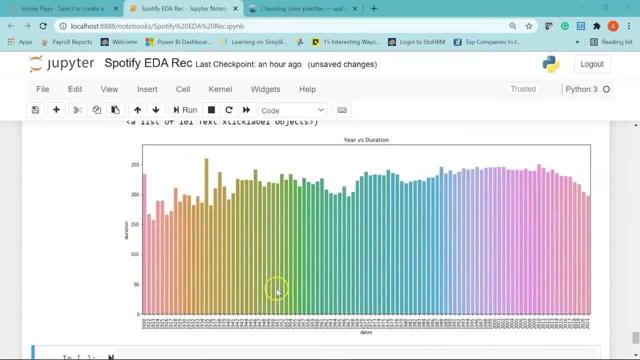 see we have the bar plot for the different years and the duration of the songs in seconds in the y-axis. so earlier in the 1920s you can see the duration of the songs were less and later it increased around late 1930s and this 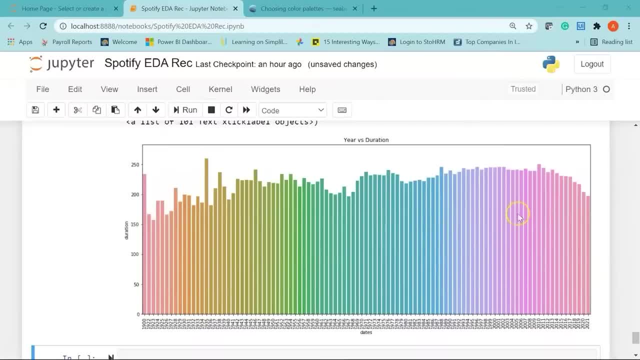 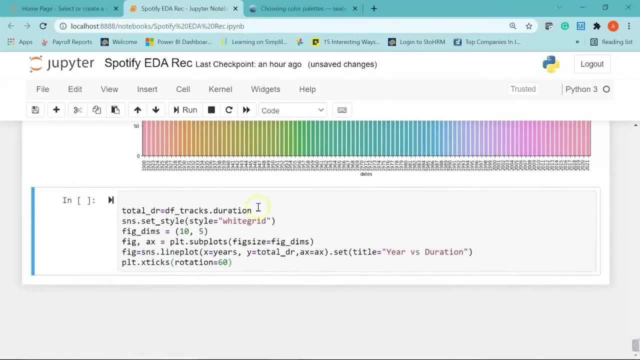 remained consistent as until 2010, where the duration was high, but after 2010 you can see the duration of the songs have started decreasing. now, in the next cell, i am going to create a line plot to analyze the average duration of the songs over the years. it is going to 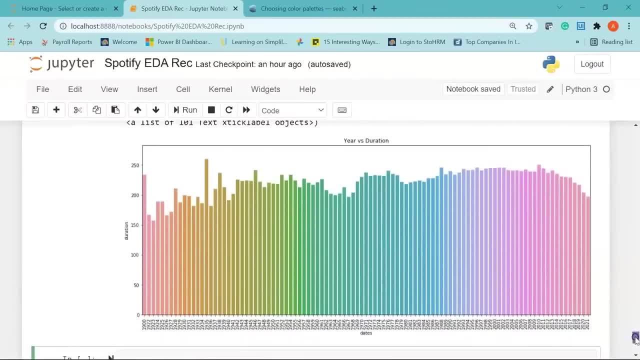 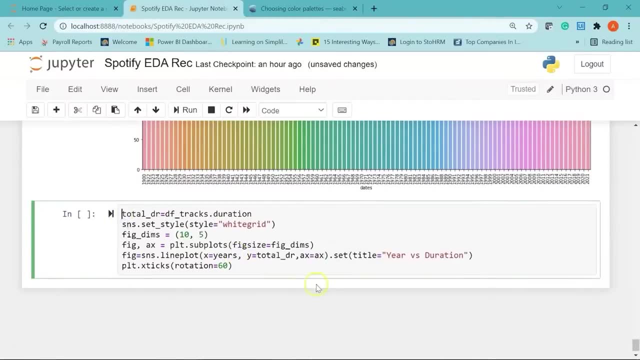 be similar to our bar plot, just that now we are going to visualize it in terms of a line plot. so i have my code ready. you can see here i have used my seaborn library and the line plot function. in the x-axis i have years and in the y-axis i have total duration. 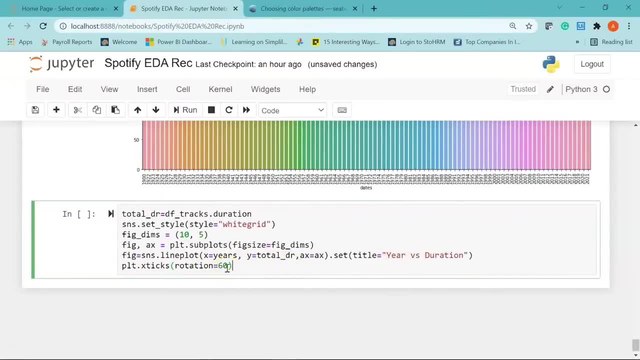 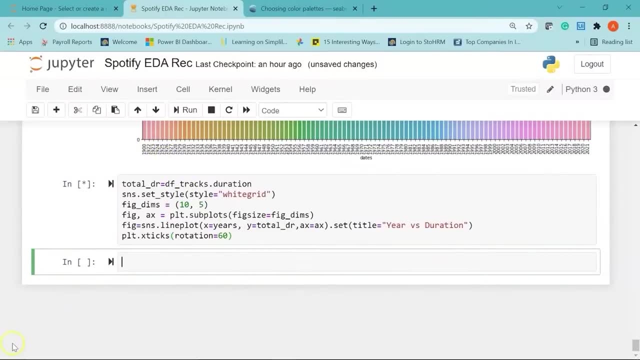 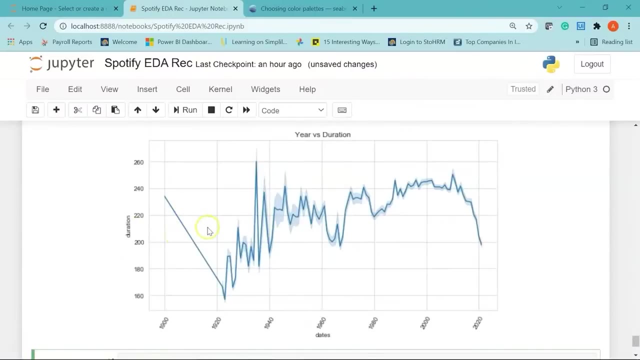 i have set my title to year versus duration and i am rotating my x labels by 60 degrees. let's run it and we will see the output. there you go now. if i scroll down, you can see line plot and on the x-axis you have the 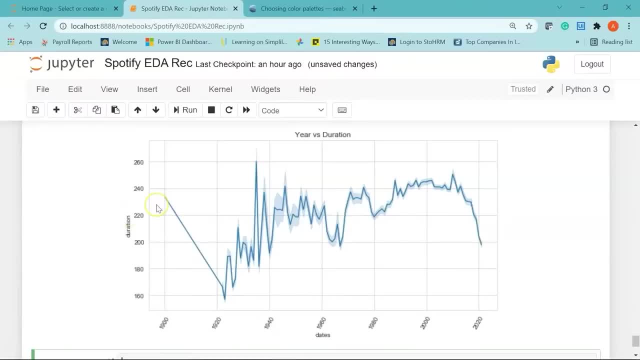 years and on the y-axis we have the duration. you can see that the songs from 1920s to 1960s have comparatively shorter duration, since most of the songs tended to be more singing based rather than instrument based. after 1960s, you can see the duration. 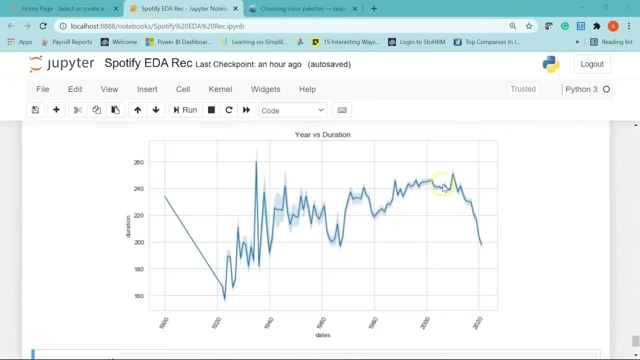 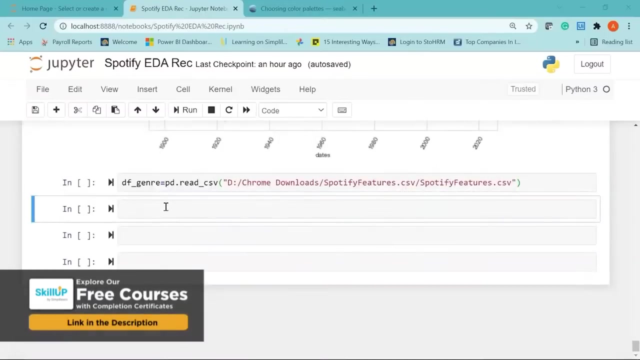 of the songs started increasing until, i would say, 2010, and, in the present day, the duration of the songs have started declining, since the attention span of the average listener is also declining. alright, now let's move to our second data analysis project, which is based on: 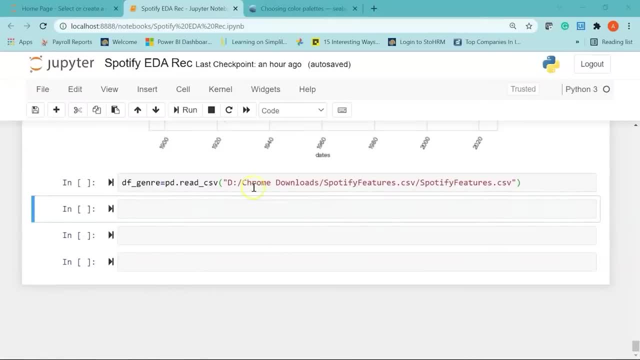 which is based on genres of the songs. So I am importing my dataset using the pandas read underscore: csv function. I have given my location and here I have my dataset name followed by the extension of the type. So this is the csv dataset. Let's go ahead and run it. 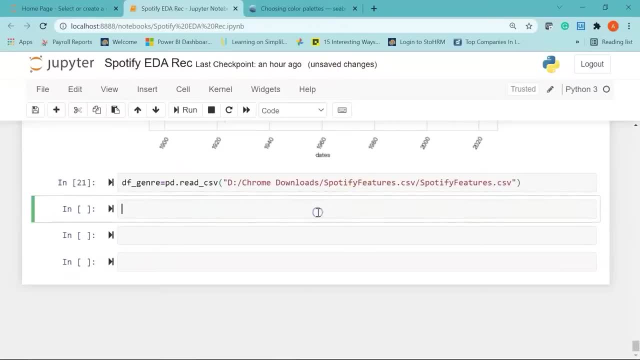 Okay, now let's print the first five rows of the dataset. I have stored my dataset in a data frame called df underscore genre. I will use the head function to get the first five rows of information. I will hit shift enter to run it. 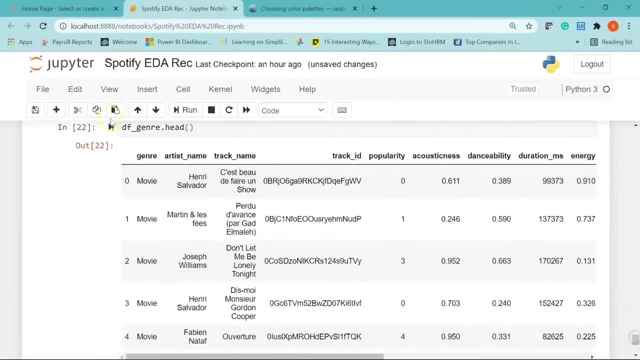 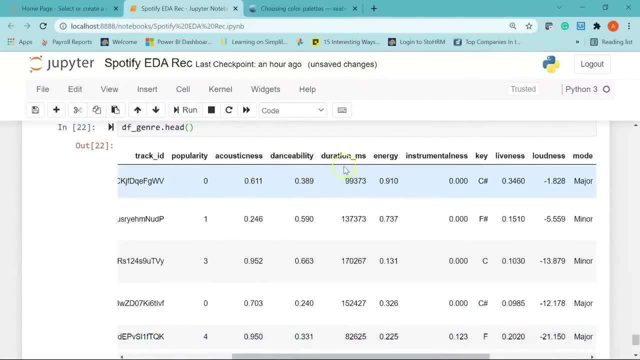 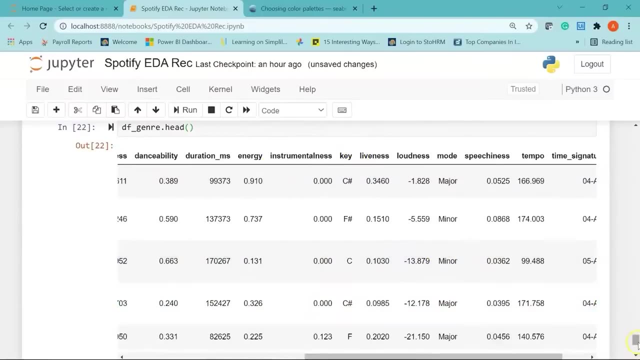 There you go. You can see here I have my genre column, artist name, track name, track id, popularity, acousticness duration in milliseconds again, and we have the rest of the other columns that we saw in our first dataset. Just one thing to note here: key. 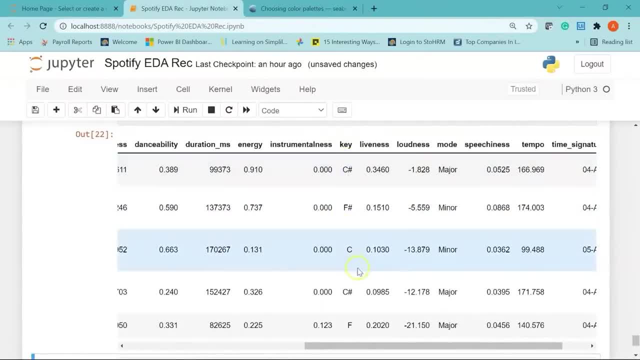 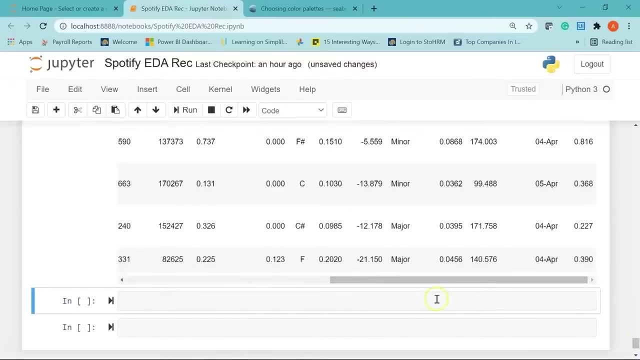 is present in terms of c, d, e, c minor, f minor, and not in terms of numbers between 0 to 11.. Now we will see the duration of the songs for different genres. For that I'm going to create a bar plot, So I'll start with. 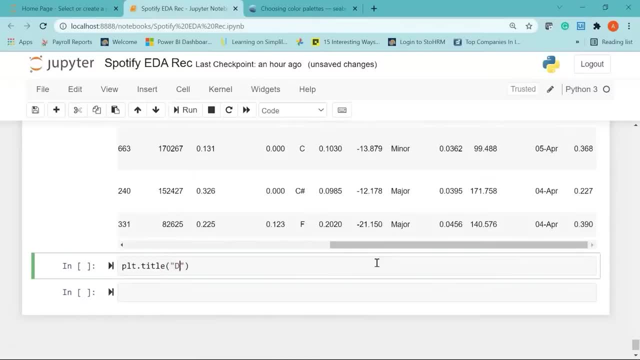 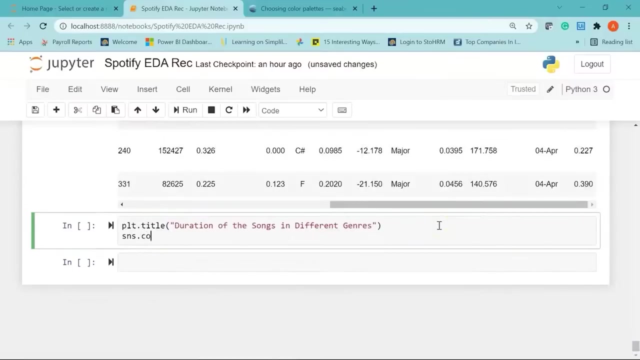 setting the title for my plot as duration of the songs in different genres, I'll use the cborn library and I'll set my color palette to, let's say, rocket into the comma and say, as cmap equal to true, This would be color palette. 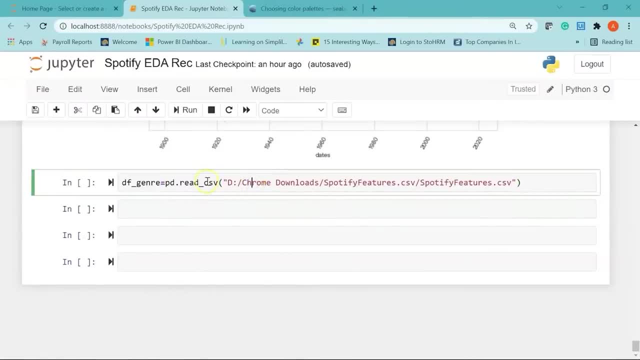 genres of the songs. so i am importing my data set using the pandas read underscore: csv function. i have given my location and here i have my data set name followed by the extension of the type. so this is the csv data set. let's go ahead and run it. 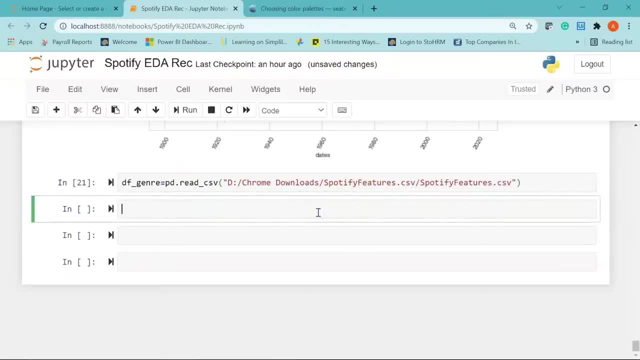 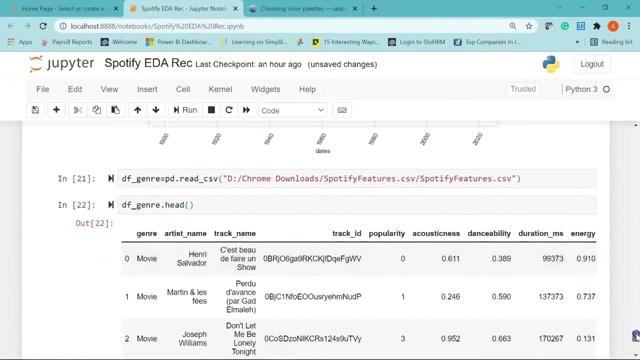 ok, now let's print the first five rows of the data set. i have stored my data set in a data frame called df underscore. i will use the head function to get the first five rows of information. i will hit shift, enter to run it. there you go. 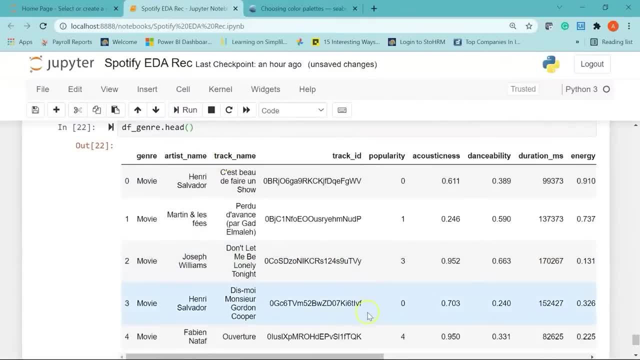 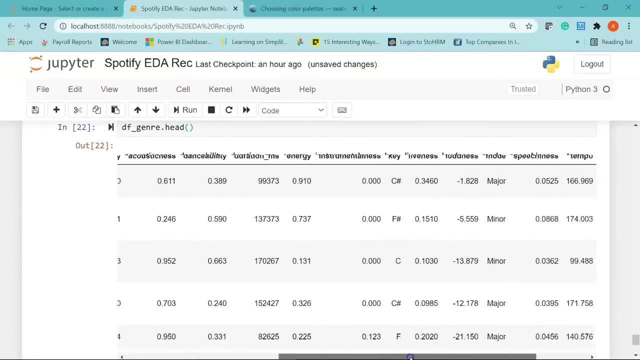 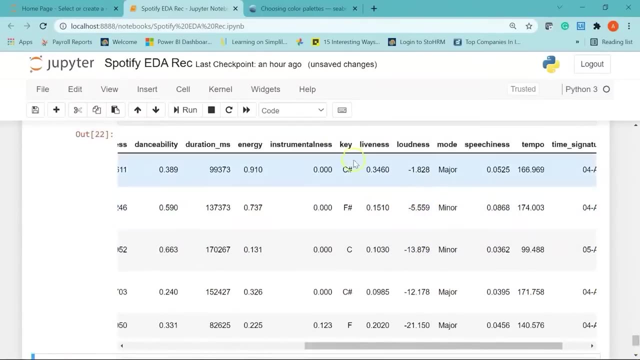 you can see here i have my genre column, artist name, track name, track id, popularity, acousticness duration in milliseconds again, and we have the rest of the other columns that we saw in our first data set. just one thing to note here: key is present in terms of c, d. 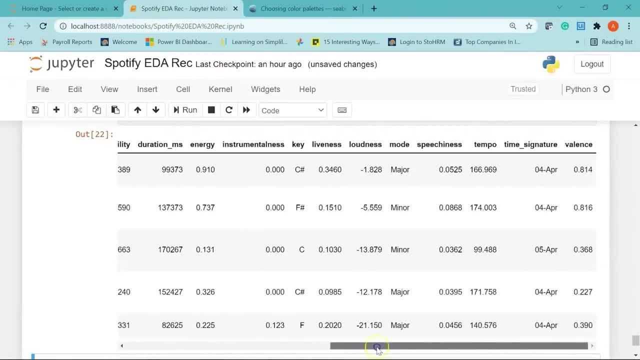 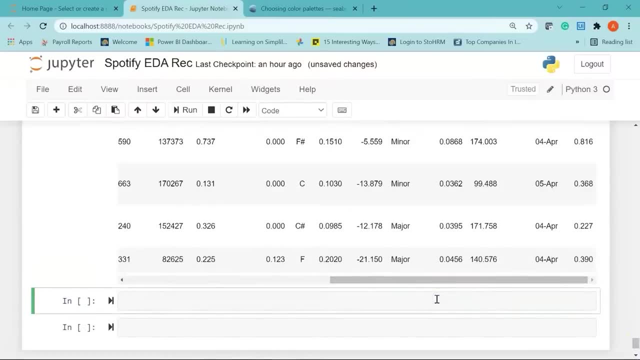 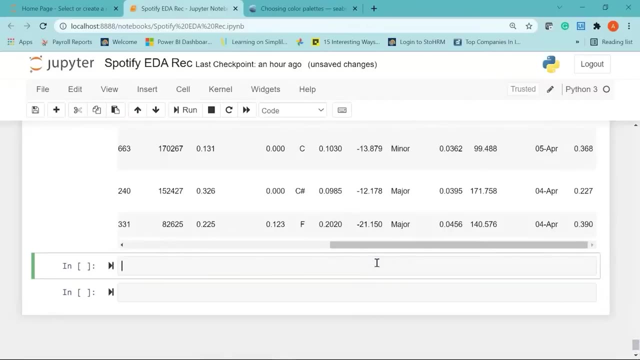 e, c minor, f minor, and not in terms of numbers between 0 to 11. now we will see the duration of the songs for different genres. for that i am going to create a bar plot, so i will start with setting the title for my plot as duration. 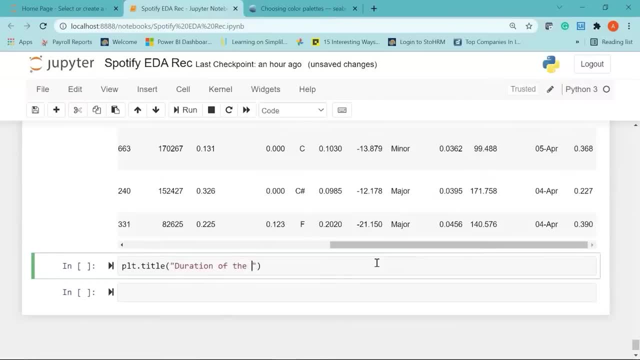 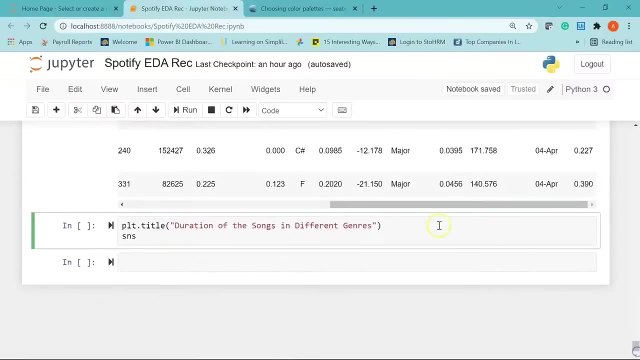 of the songs and in different genres. i will use the seaborn library and i will set my color palette to, let's say, rocket into the comma and say as c map equal to true, this would be color palette. now i will say sns dot bar plot in the y axis. 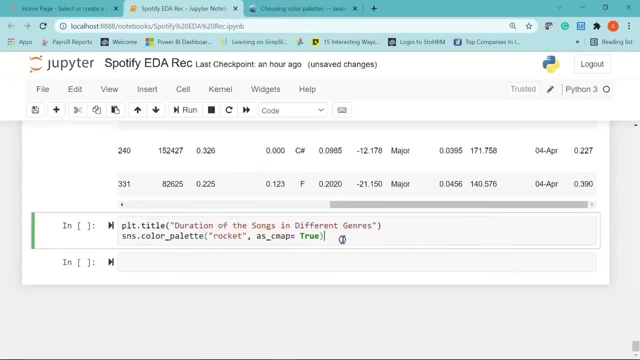 Now I'll say sns dot, bar plot, in the y-axis I'll have genre and in the x-axis I'll have my duration column, which is in milliseconds, So duration underscore ms. and then I pass my data frame using the data argument, So I'll say data equal to df dot. 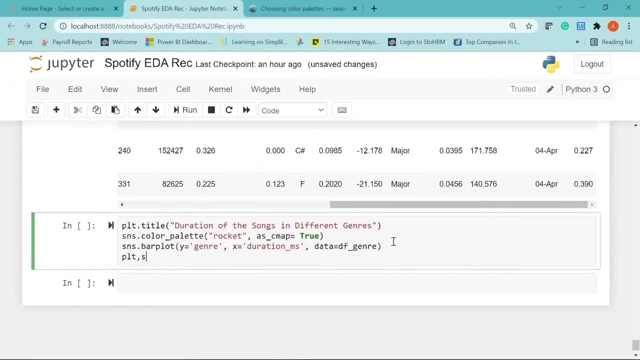 genre. Next we'll set the x labels. So I'll say plt, dot, x label. Let's say my x label is duration in milliseconds. And then I'll say I'll say plt, dot, y label as genres. Now let's go ahead and 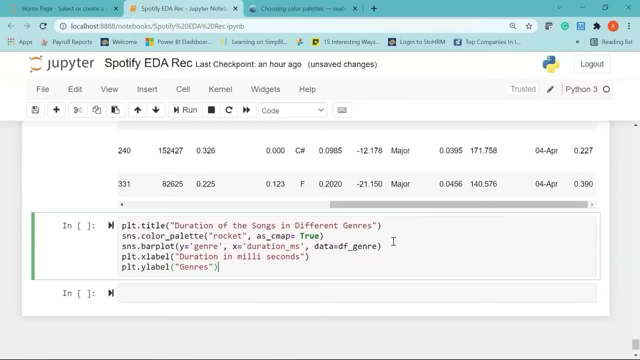 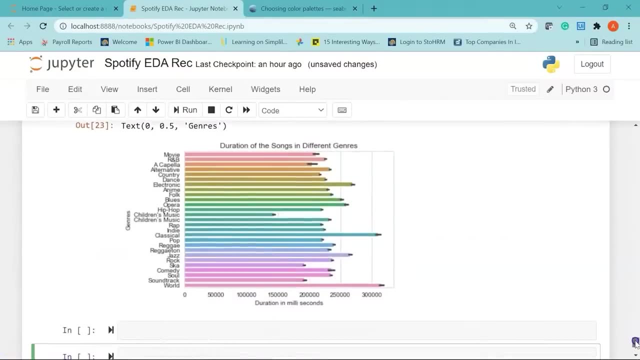 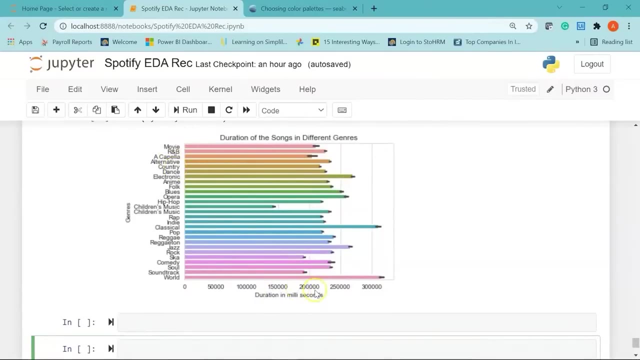 run this. There you go. So here you can see we have the different genres on the y-axis and on the x-axis. you have the duration in milliseconds And if you see the graph for classical genre and for songs that belong to world genre, the duration of the songs. 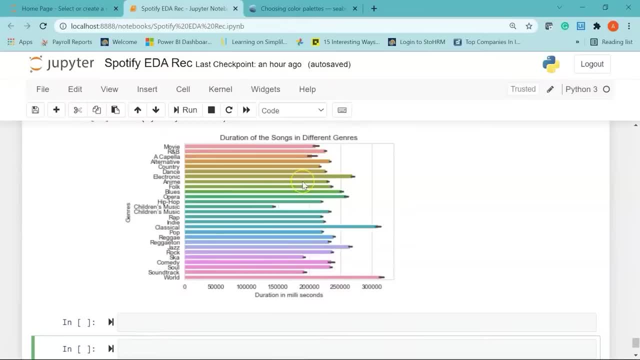 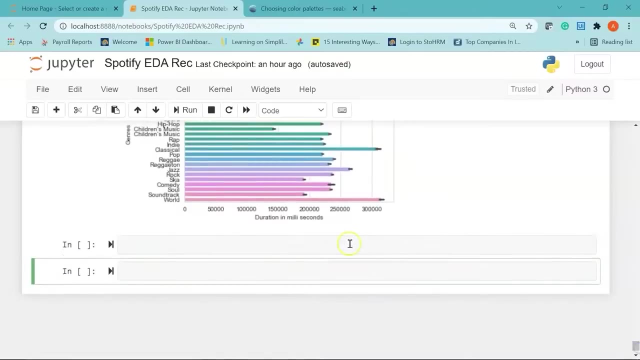 are more compared to other genres. Now, if you check for children's music genre, the duration is less or the least cool. And finally we'll move to our last demo, where we'll see the top five genres by popularity. So I'll say sns dot. 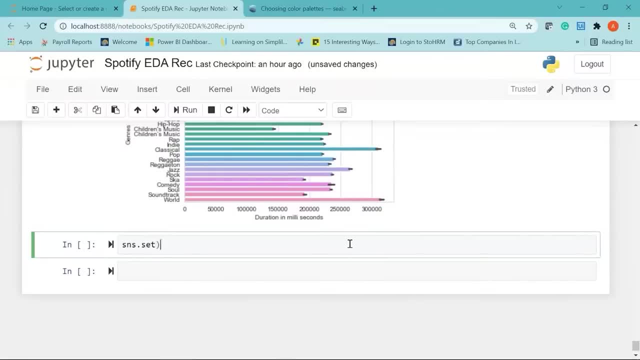 set underscore style. I'll set my style to dark grid, which will be my background, And then I'll say plt, dot figure. I'll set my figure size to 10 comma 5.. Then I'll create a variable called famous, since I want to take 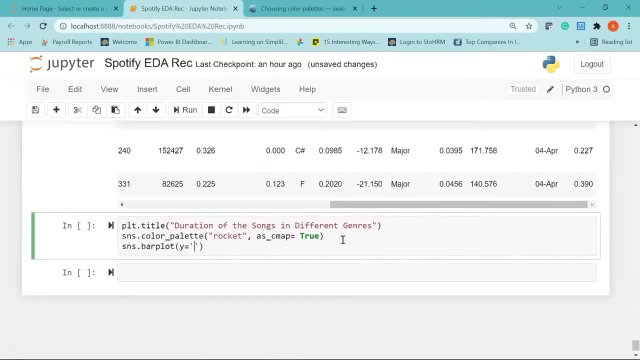 i will have genre and in the x axis i will have my duration column, which is in milliseconds, so duration underscore ms, and then i pass my data frame using the data argument, so i will say data equal to df, dot, genre. next we will set the x labels. 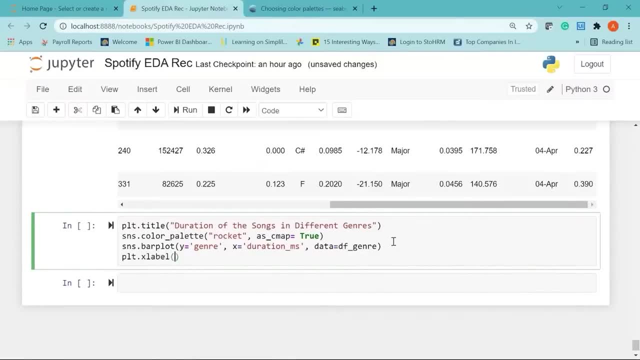 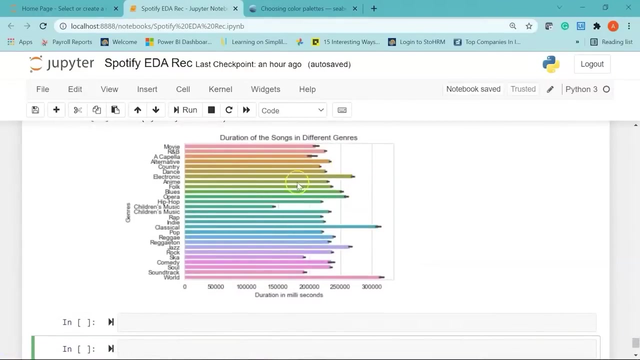 so i will say plt dot x label. let's say my x label is duration in milliseconds, and then i will say plt dot y label as genres. now let's go ahead and run this. there you go. so here you can see, we have the different genres on the y axis and 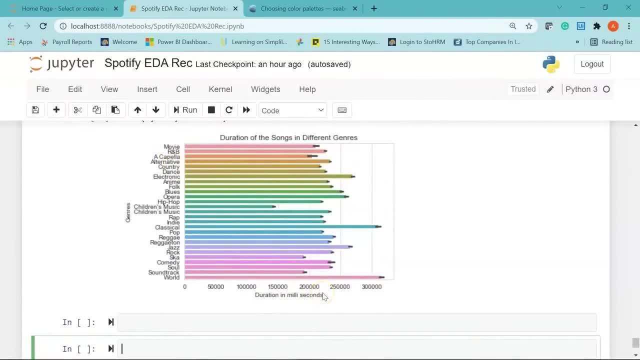 on the x axis you have the duration in milliseconds and if you see the graph for classical genre and for songs that belong to world genre, the duration of the songs are more compared to other genres. now, if you check for children's music genre, the duration is less. 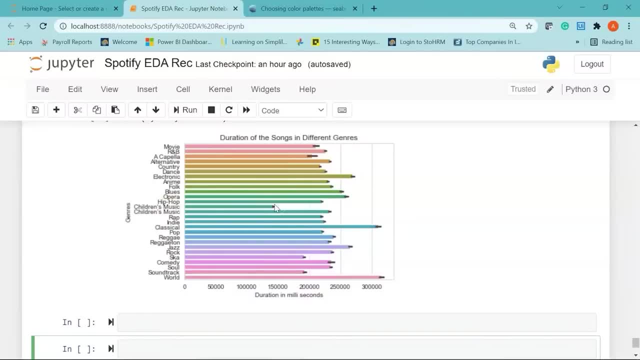 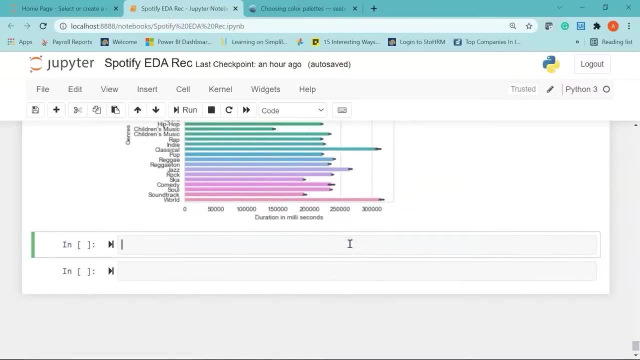 or the least cool. and finally, we will move to our last demo, where we will see the top five genres by popularity. so i will say: sns dot, set underscore style. i will set my style to dark grid, which will be my background, and then i will say: plt dot. 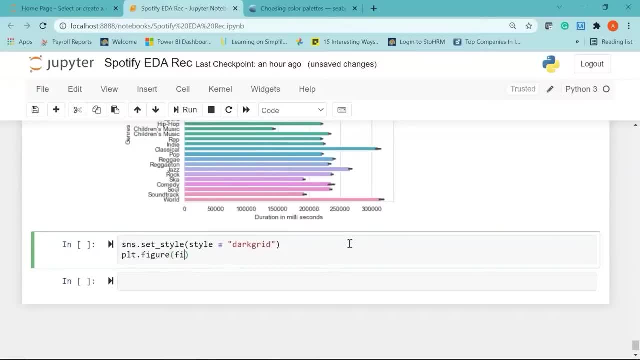 figure. i will set my figure size to 10 comma 5, then i will create a variable called famous, since i want to take only the most popular songs based on the genre. so i have created a variable called famous and i will pass my data frame name, that is df underscore. 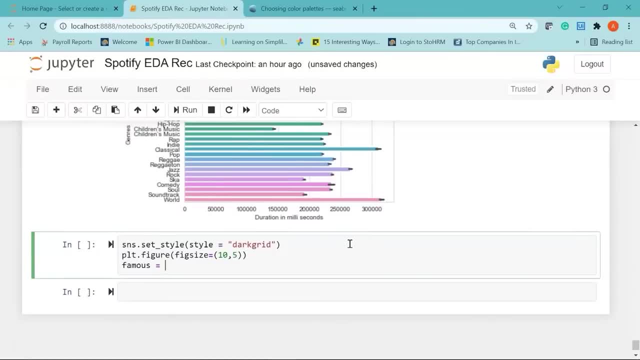 only the most popular songs based on the genre. So I have created a variable called famous and I'll pass my data frame name, that is df, under the score genre and I'll sort the values based on my popularity column. So I'll say popularity and I want to. 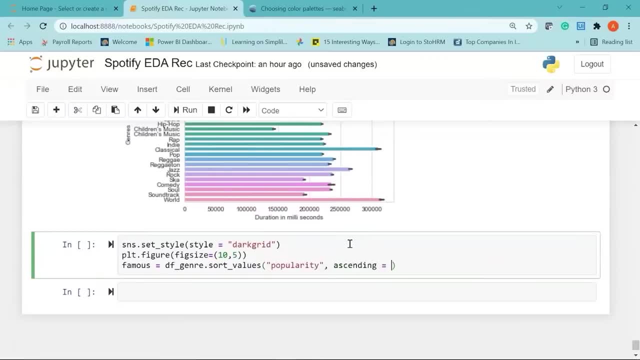 sort it in descending order. So I'll say ascending equal to false and I'll take the first 10 values. I'll tell you the reason why I'm taking the first 10 values and not 5.. Then I'll say sns dot barplot. 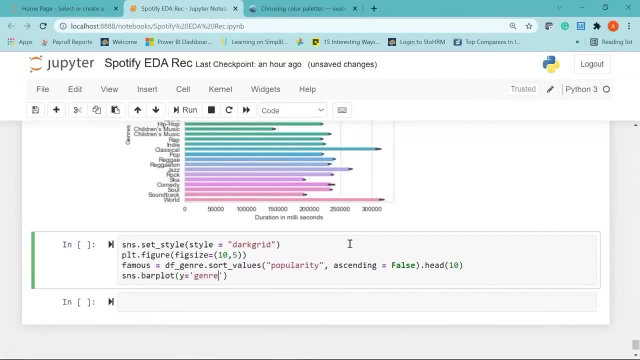 and in the y-axis I'll have genre, In the x-axis we'll have popularity, and I'll give a comma and, using the data argument, I'll say my data to be famous, which is this variable that we created, and then I'll set my title. 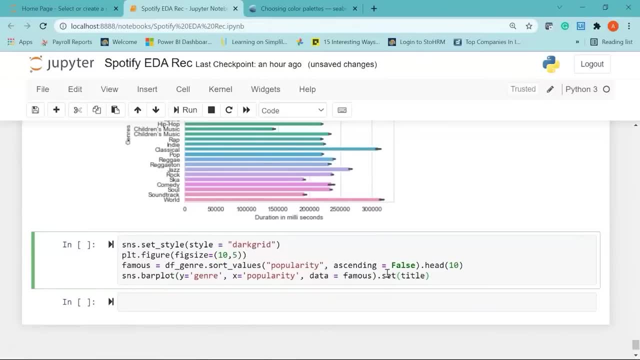 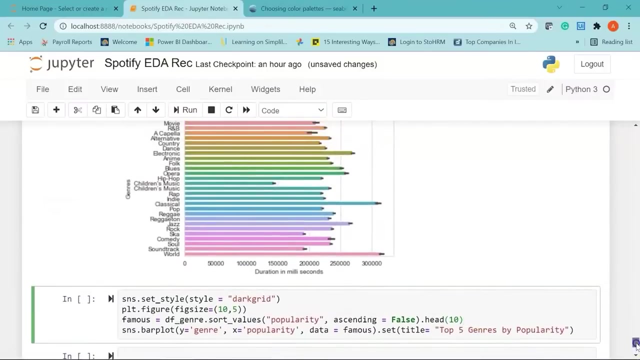 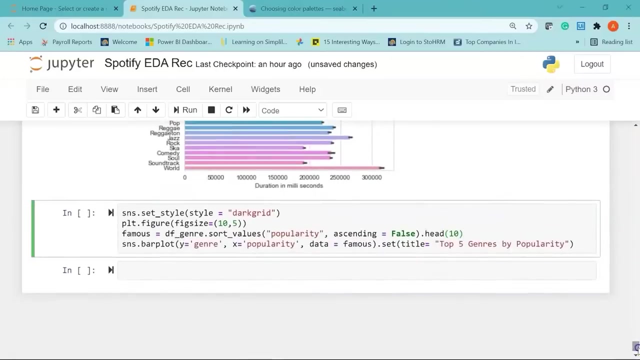 as top 5 genres by popularity. Alright. Now, the reason why I took head of 10 is because there are a few genres which are repetitive. So, if you see this, we have children's music appearing twice, So hence we have taken 10. 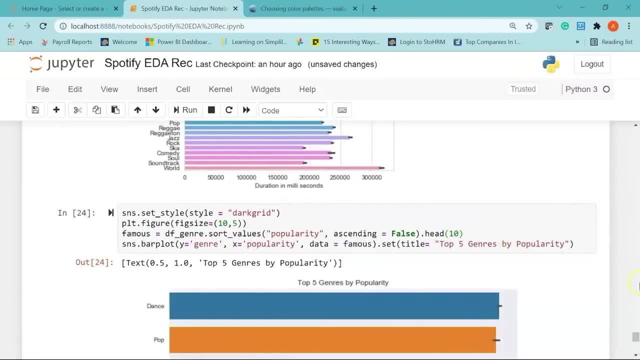 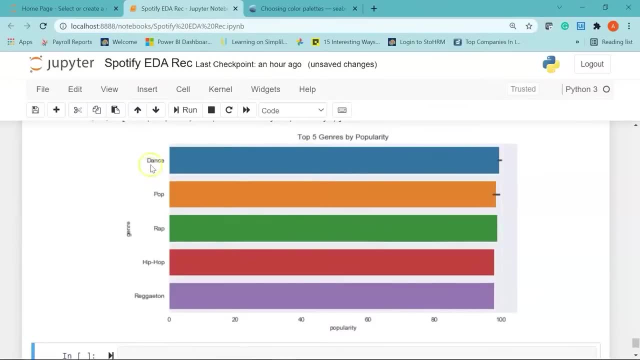 instead of 5.. Let me just go ahead and run it. There you go. So here, if I scroll down, you can see I have my top 5 genres based on the popularity. So we have dance, pop, rap, hip-hop and reggaeton. 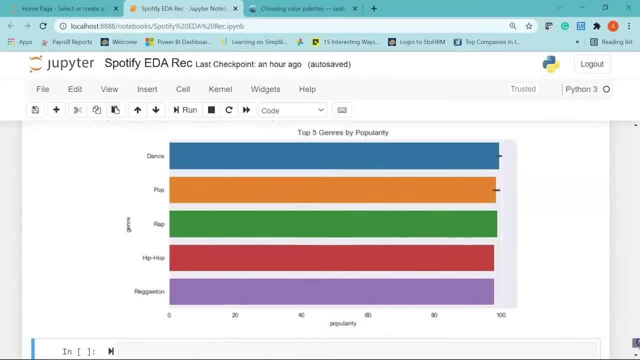 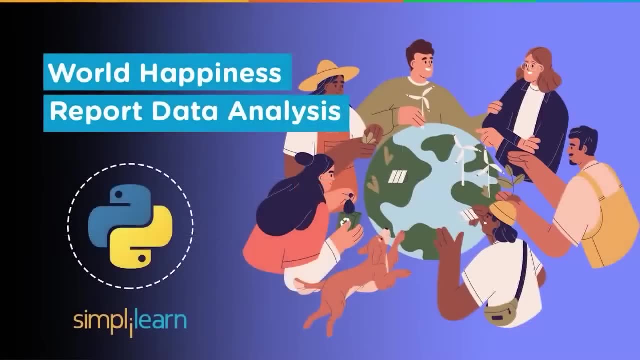 So these are the 5 genres which are most popular, based on the data that we have collected from Spotify. Alright, Hi everyone. Welcome to this really interesting video on data analysis of the 2021 world happiness report using Python. So today we will perform some exploratory. 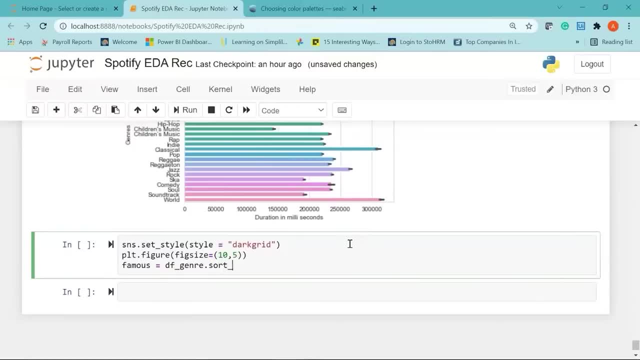 genre and i will sort the values based on my popularity column. so i will say popularity and i want to sort it in descending order, so i will say ascending equal to false and i will take the first 10 values. i will tell you the reason why i am taking the 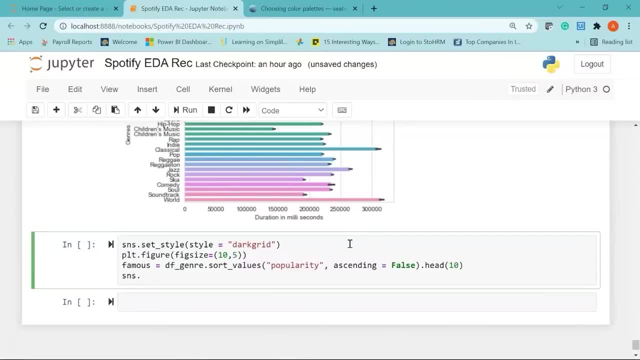 first 10 values and not 5. then i will say sns, dot, bar, plot and in the y-axis i will have genre, in the x-axis we will have popularity and i will give a comma and, using the data argument, i will say my data to be: 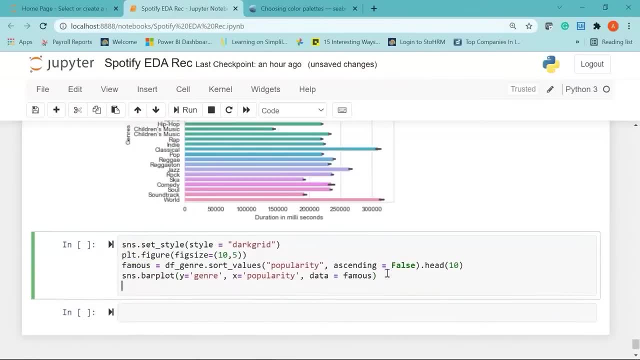 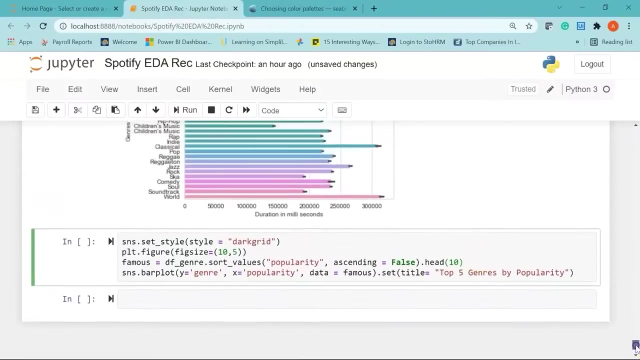 famous, which is this variable that we created, and then i will set my title as top five genres by popularity. alright, now, the reason why i took head of 10 is because there are a few genres which are repetitive. so, if you see this, we have children's music. 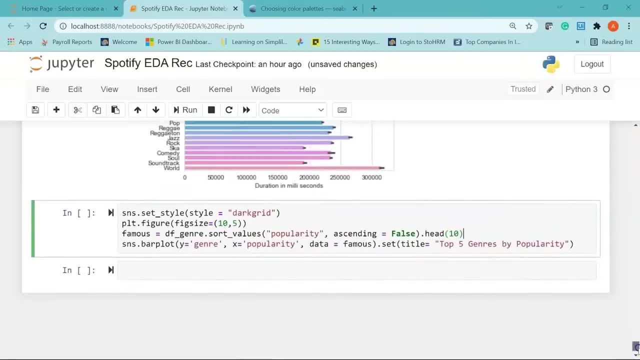 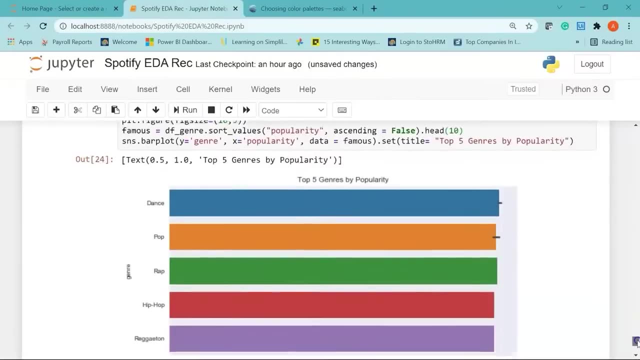 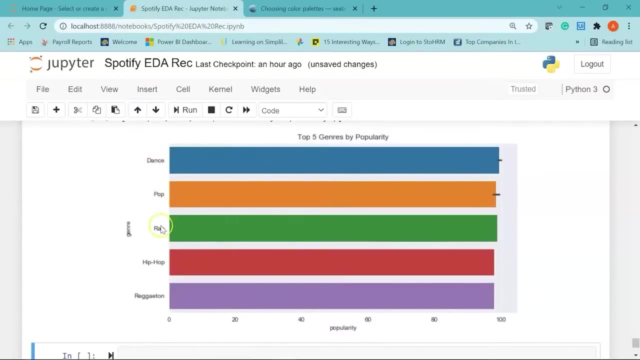 appearing twice, so hence we have taken 10 instead of 5. let me just go ahead and run it. there you go. so here, if i scroll down, you can see i have my top five genres based on the popularity. so we have dance, pop, rap, hip-hop and reggaeton. 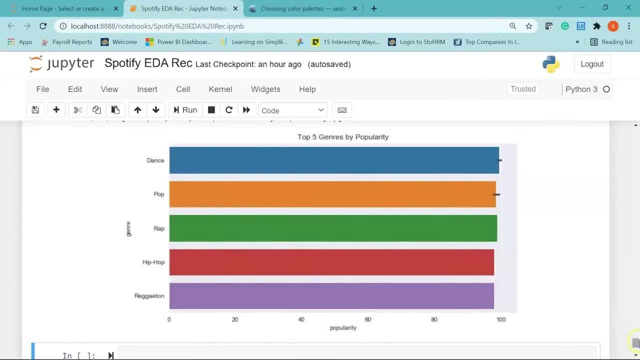 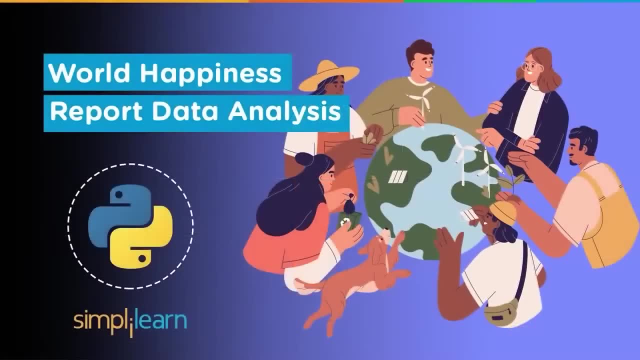 so these are the five genres which are most popular, based on the data that we have collected from spotify. alright, hi everyone. welcome to this really interesting video on data analysis of the 2021 world happiness report using python. so today we will perform some exploratory data analysis using python. 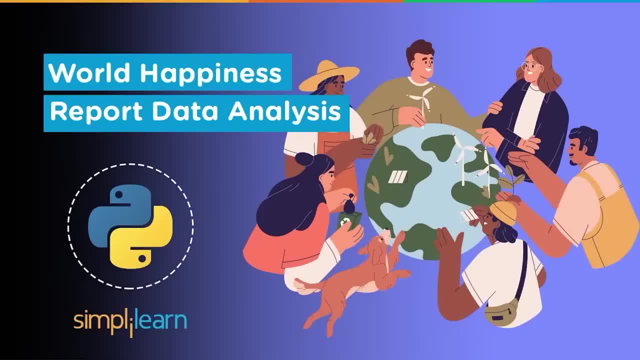 libraries to analyze, visualize and draw insights from 2021 world happiness data. before i begin, make sure to subscribe to the simply lon channel and hit the bell icon to never miss an update. first, let's understand what the world happiness report 2021 is all about. 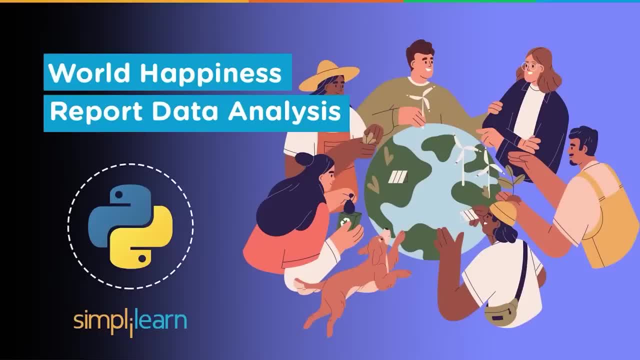 data analysis using Python libraries to analyze, visualize and draw insights from 2021 world happiness data. Before I begin, make sure to subscribe to the SimplyLoan channel and hit the bell icon to never miss an update. First, let's understand what the world happiness report. 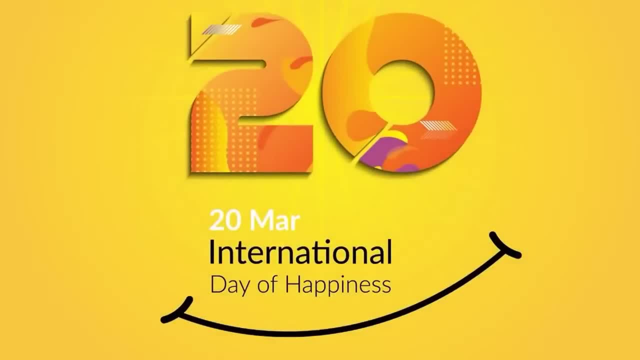 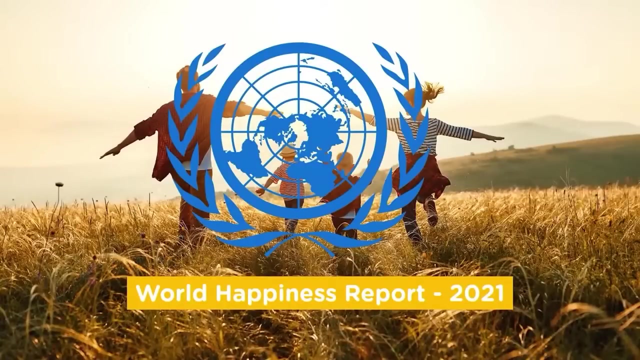 2021 is all about. The International Happiness Day is celebrated every year since 2013 on 20th of March to emphasize the importance of happiness in the daily lives of people. So the United Nations Sustainable Development Solutions Network published the world happiness report on 19th of March 2021. 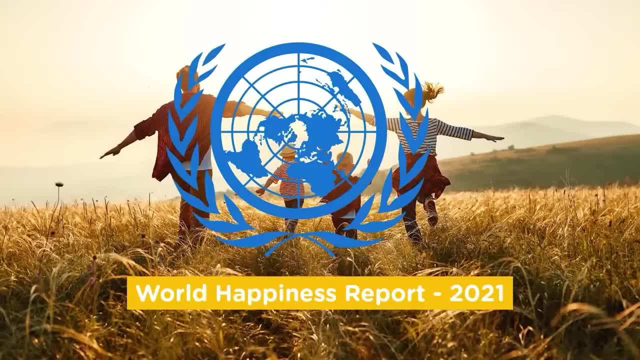 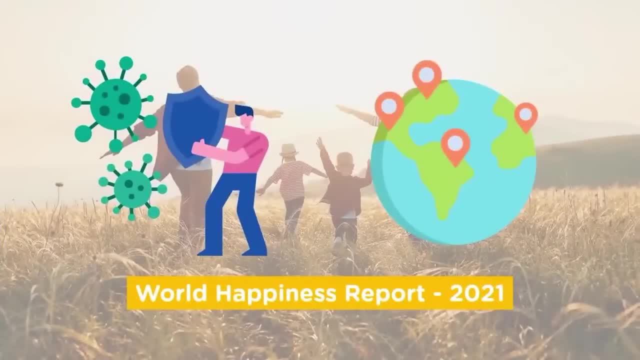 that ranks the world's 149 countries on how happy the citizens perceive themselves to be, based on various indicators. The happiness study ranks the countries on the basis of questions from the Gallup World Poll. The results are then equated with other factors such as GDP. 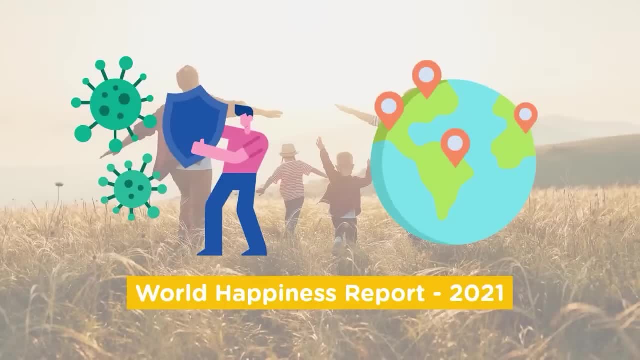 life expectancy, generosity, etc. This year, it focused on the effects of the COVID-19 pandemic and how people all over the world have managed to survive and prosper. So, using this 2021 data, we will answer critical questions such as the top 10. 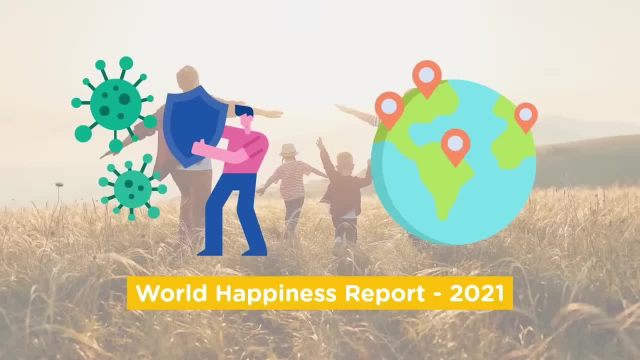 most corrupt countries. We will plot a graph to understand how the happiness score is related to the freedom of making life choices. We will look at the life expectancy of 10 happiest and 10 least happy nations. So these are a few examples, but we will explore more about the data. 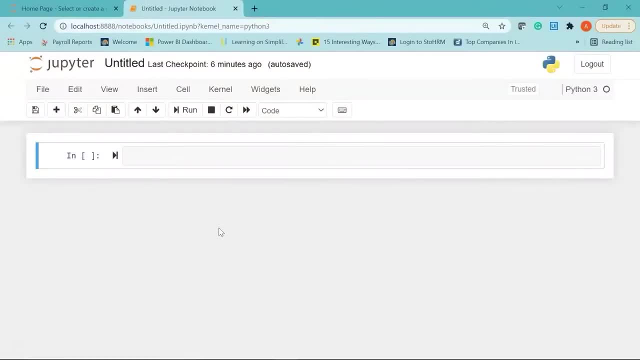 in detail in our demo session. Let's get started. So first I will show you the data set we will be using in this demo. So this data has been collected from Kegel. Let me show you that. So this is the CSB. 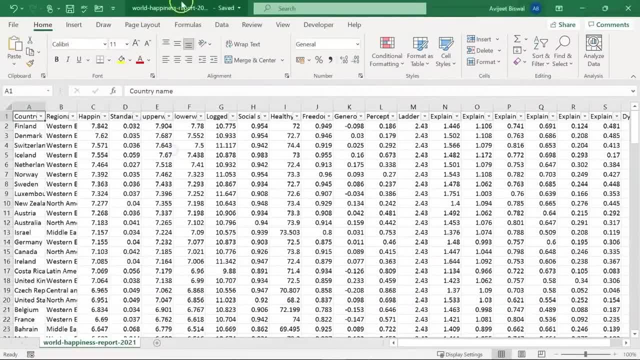 data set that we have downloaded from kegelcom So you can see here world happiness report 2021 and we will share the data set link in the description of the video You can click on the link to download the data set. Now we have information about 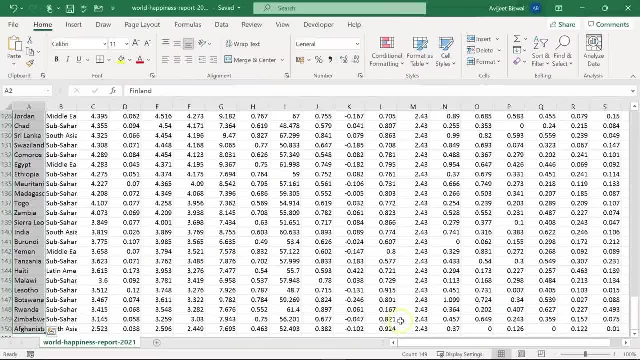 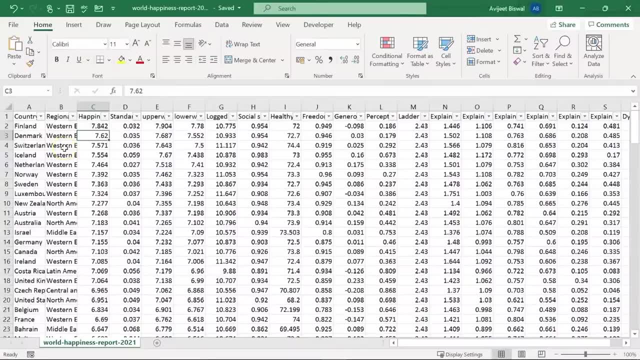 149 countries. You can see it here. Count is 149.. Let me go to the top and I will run through the columns that are there in this data set. So the first column is the country name. So we have 149 different countries. 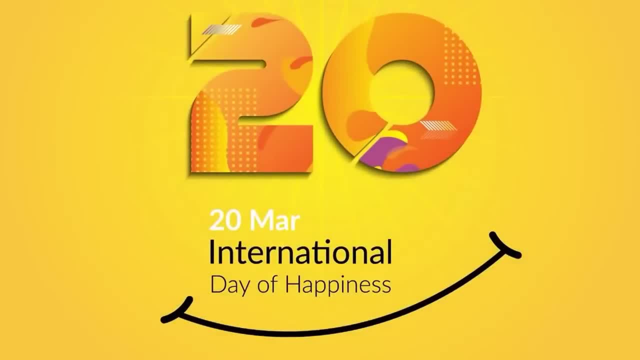 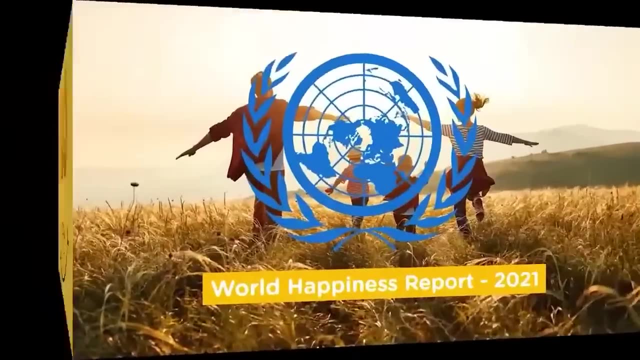 the international happiness day is celebrated every year since 2013 on 20th of march, to emphasize the importance of happiness in the daily lives of people. so the united nations sustainable development solutions network published the world happiness report on 19th of march 2021. 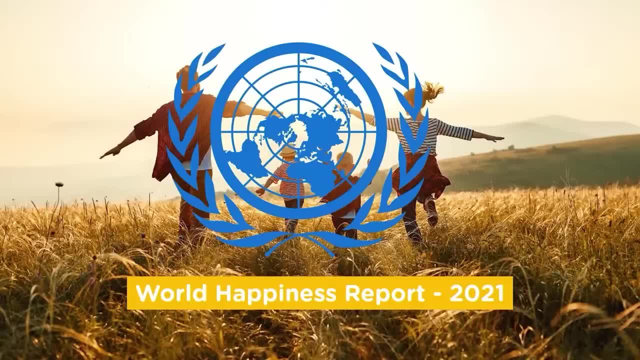 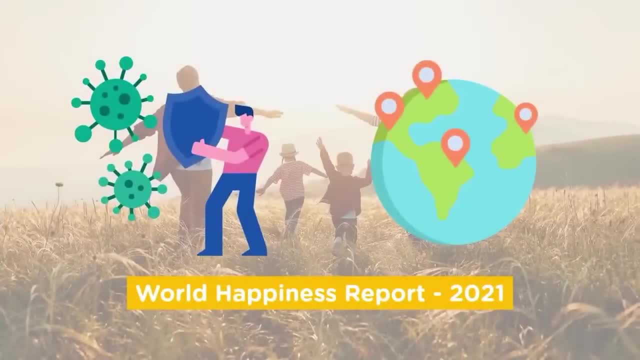 that ranks the world's 149 countries on how happy the citizens perceive themselves to be, based on various indicators. the happiness study ranks the countries on the basis of questions from the gallup world poll. the results are then equated with other factors such as gdp. 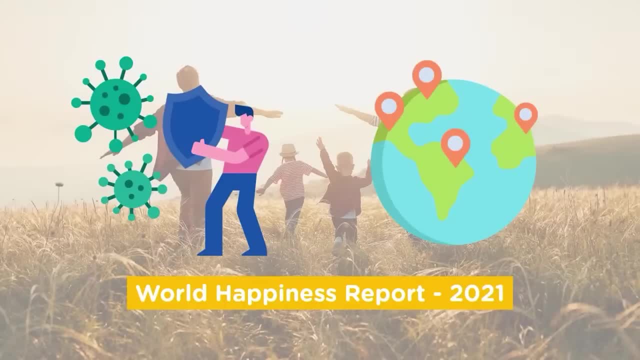 life expectancy, generosity, etc. this year, it focused on the effects of the covid 19 pandemic and how people all over the world have managed to survive and prosper. so, using this 2021 data, we will answer critical questions such as the top 10 most corrupt countries. 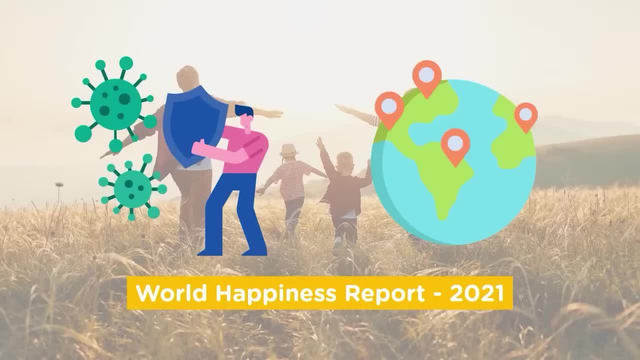 we will plot a graph to understand how the happiness score is related to the freedom of making life choices. we'll look at the life expectancy of 10 happiest and 10 least happy nations. so these are a few examples, but we will explore more about the data. 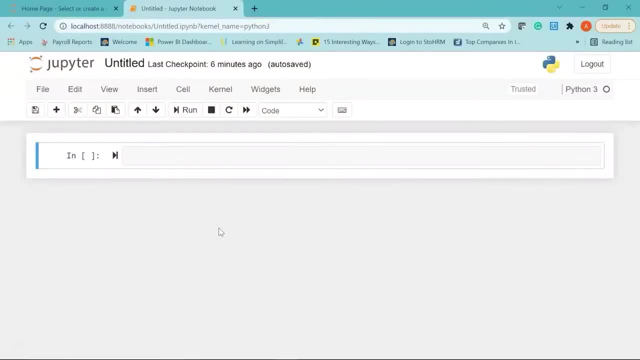 in detail in our demo session. let's get started. so first i'll show you the data set we'll be using in this demo. so this data has been collected from kegel. let me show you that. so this is the csv data set that we have downloaded from. 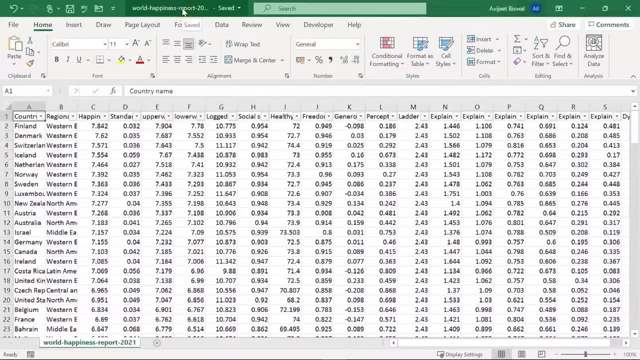 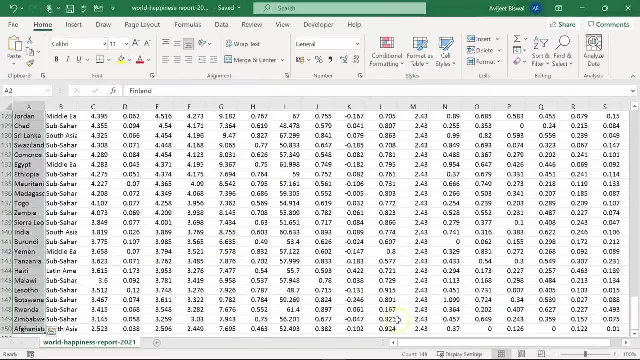 kegelcom so you can see here world happiness report 2021 and we will share the data set link in the description of the video. you can click on the link to download the data set now we have information about 149 countries. you can see it here. 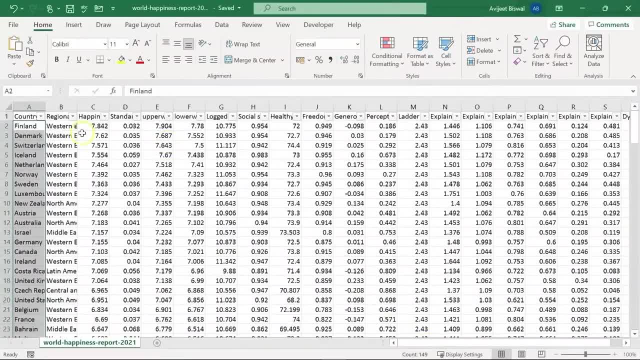 count is 149. let me go to the top and i'll run through the columns that are there in this data set. so the first column is the country name. so we have 149 different countries, and then we have something called as regional indicator. we can call this as just the region. 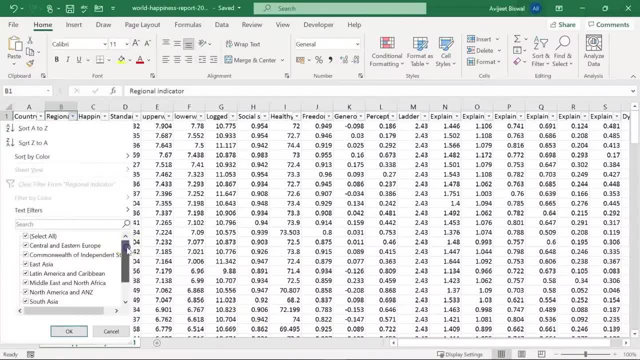 so you can see we have different regions. i've applied a filter. we have central and eastern europe, then we have commonwealth of independent states, so these include countries such as russia. then we have east asia, latin america and caribbean. we also have south asia, south east asia, sub-saharan. 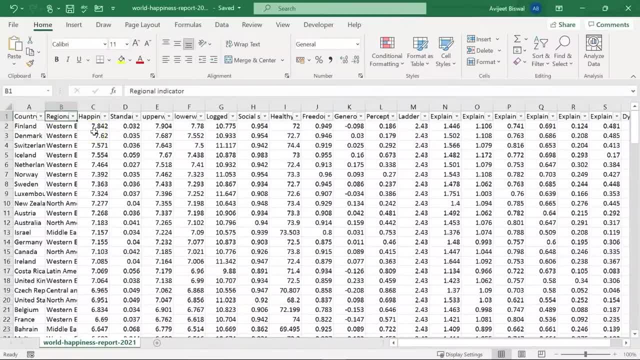 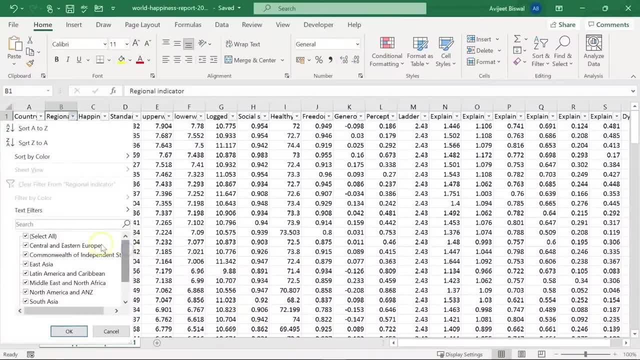 and then we have something called as regional indicator. You can call this as just the region, So you can see we have different regions. I have applied a filter. We have Central and Eastern Europe. Then we have common wealth of independent states, So these include countries such 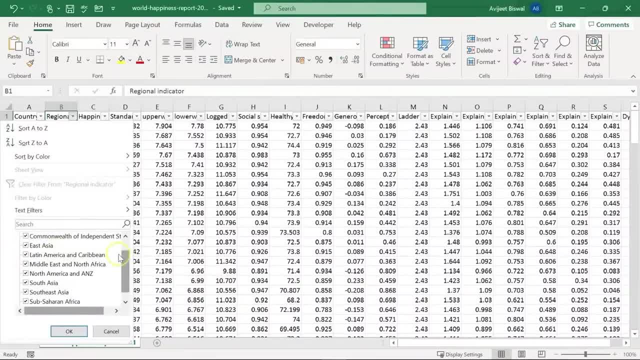 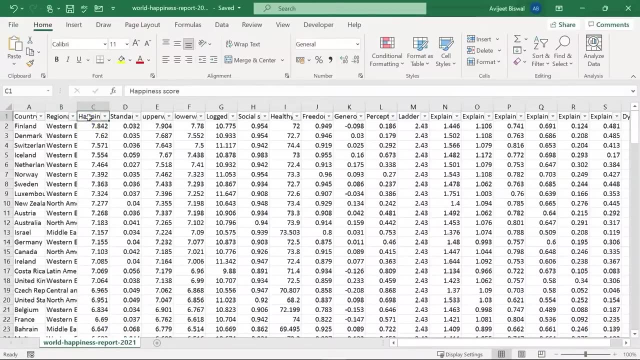 as Russia. Then we have East Asia, Latin America and Caribbean. We also have South Asia, Southeast Asia, Sub-Saharan Africa, Western Europe and other regions. I will just cancel this. And then we have the happiness score column. that has been sorted in descending order. 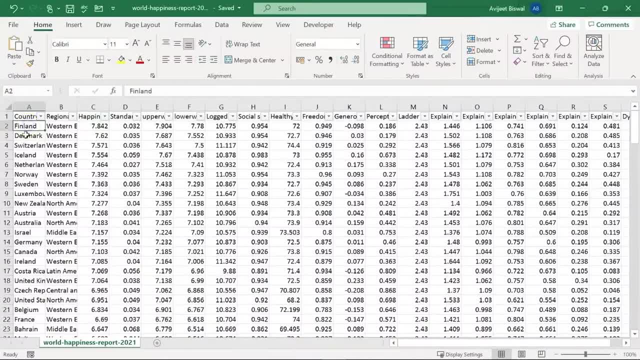 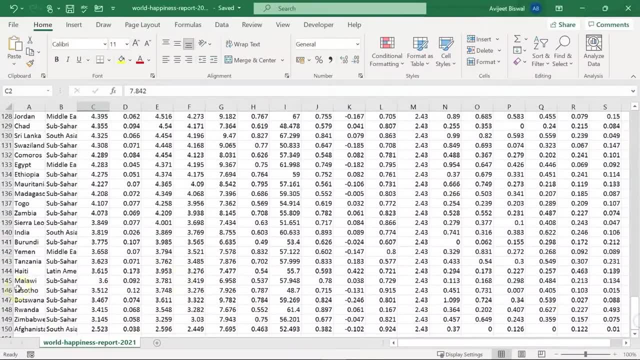 So we have Finland, Denmark and Switzerland, who are the top three happiest nations. Now, if I scroll down, we have countries like Rwanda, Zimbabwe and Afghanistan, which are the least three happy countries. Now there are a few columns that we won't be using in. 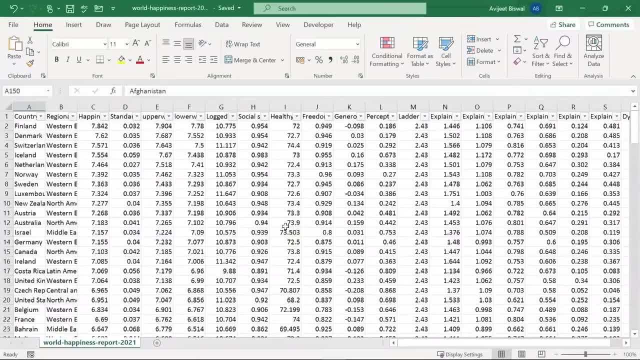 our analysis. So we will learn how to exclude those columns and keep only the relevant ones, So columns such as standard error of ladder score. Then we have upper whiskers and lower whisker column. So we are going to ignore these columns, We are only concerned. 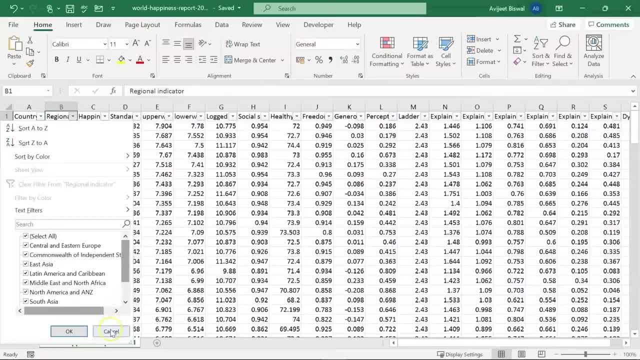 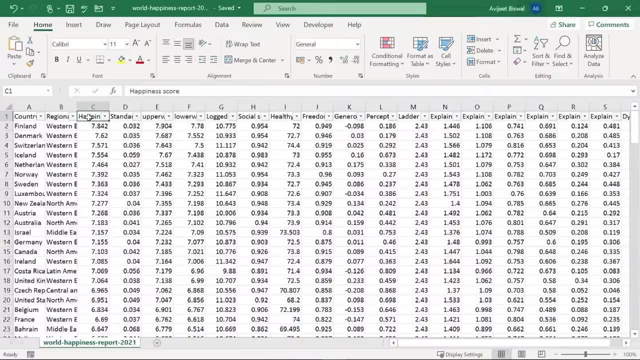 africa, western europe and other regions. i'll just cancel this. and then we have the happiness score column. that has been sorted in descending order, so we have finland, denmark and switzerland, who are the top 3 happiest nations. now, if i scroll down, we have countries like: 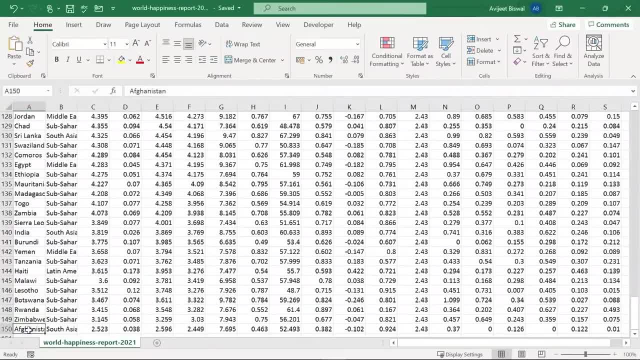 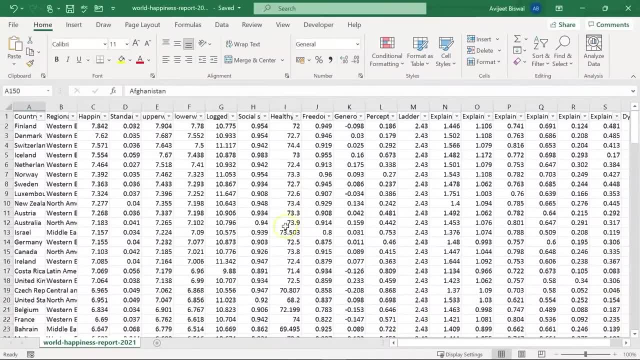 Rwanda, Zimbabwe and Afghanistan, which are the least 3 happy countries. now there are a few columns that we won't be using in our analysis, so we will learn how to exclude those columns and keep only the relevant ones. so columns such as standard error of ladder score. then we have 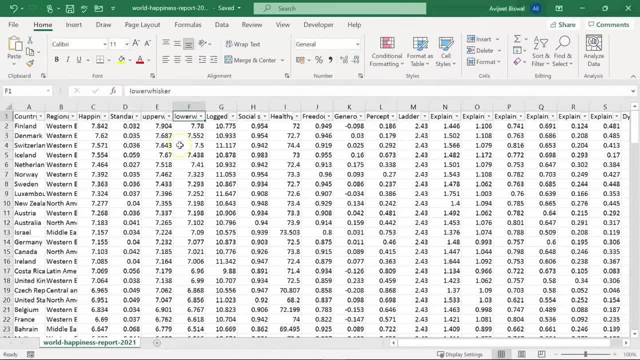 upper whiskers and lower whisker column. so we are going to ignore these columns. we are only concerned about the GDP column, which is this one. then we have the social support or the social status column. then we have the health, life expectancy, freedom to make life choices, generosity. 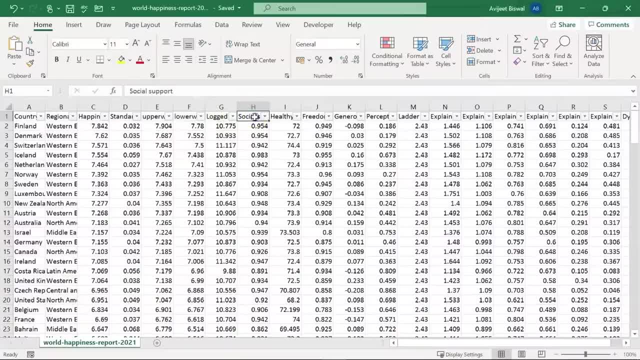 about the GDP column, which is this one. Then we have the social support or the social status column. Then we have the health, life expectancy, freedom to make life choices, generosity and perceptions of corruption, And there are a few other columns you can see to the right and 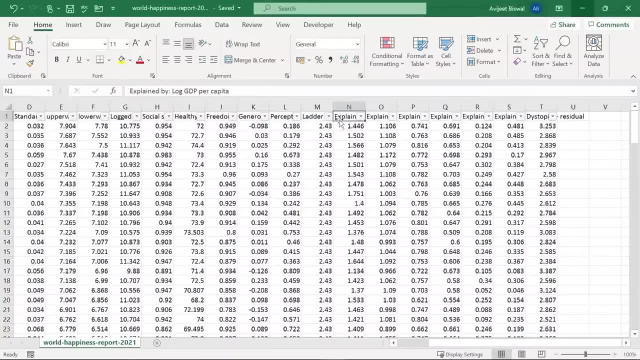 these columns are not of our interest, So we are going to ignore them. Now let's head over to our Jupiter notebook, and we will start by importing all the necessary libraries for analysis and data visualization. Okay, so I am on my Jupiter notebook, So first step, I will 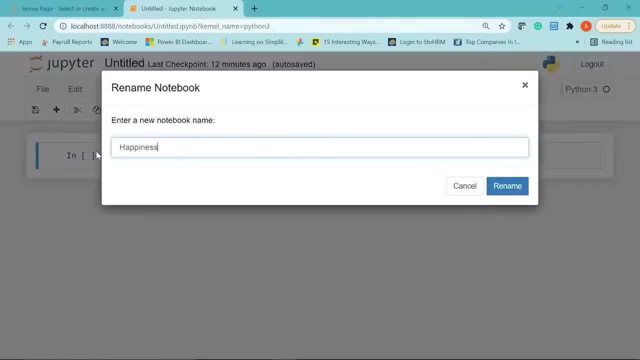 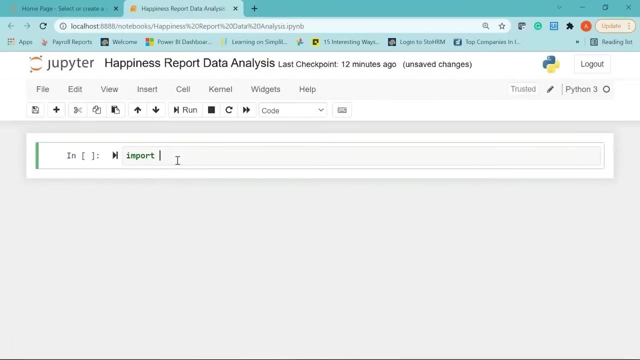 just rename this notebook to, let's say, happiness report data analysis. I will click on rename Alright. Now we will start by importing our libraries. So first library I am going to import is numpy as np. Then I have import pandas as pd. 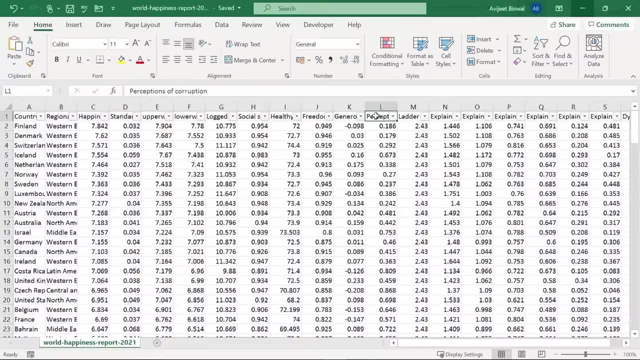 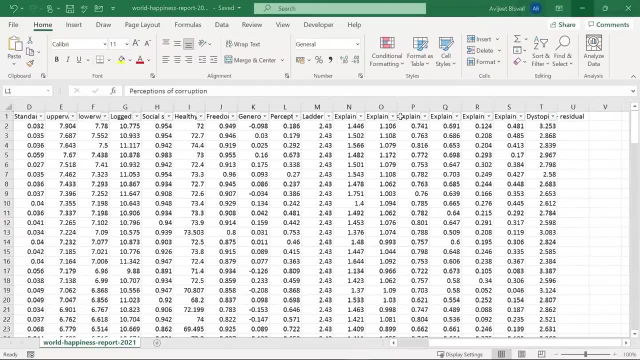 and perceptions of corruption, and there are a few other columns you can see to the right, and these columns are not of our interest, so we are going to ignore them. now let's head over to our jupiter notebook, and we will start by importing all the necessary libraries for analysis. 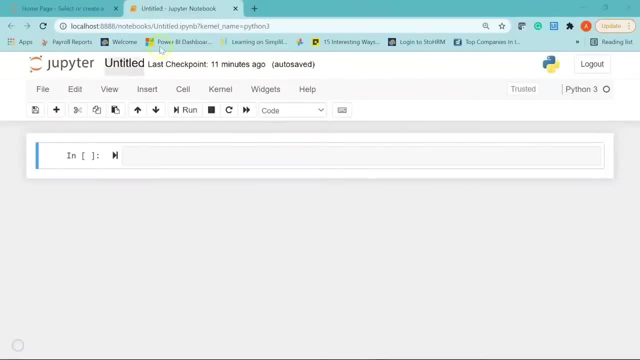 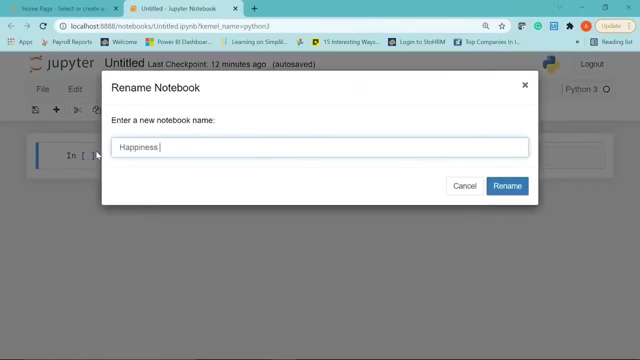 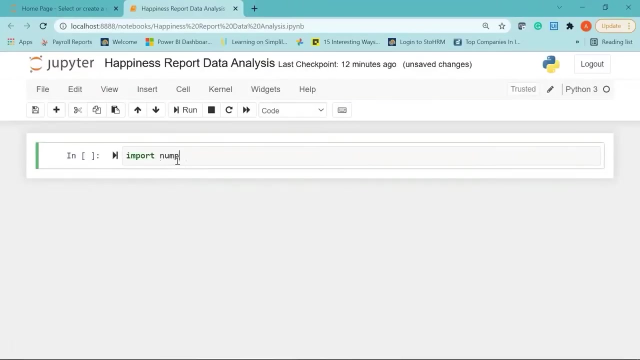 and data visualization. okay, so i am on my jupiter notebook. so first step, i will just rename this notebook to, let's say, happiness report, data analysis. i will click on rename alright. now we will start by importing our libraries. so first library i am going to import is numpy. 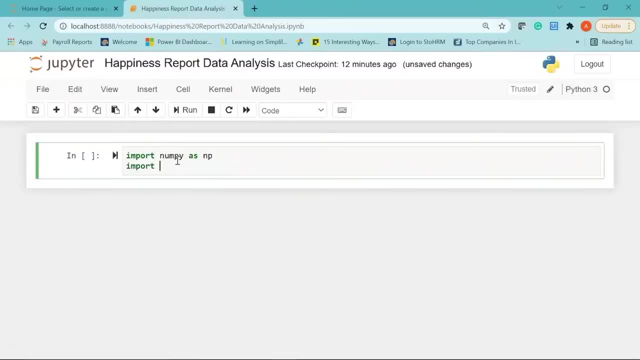 as np, then i have import pandas as pd, then i will import two data visualization libraries, seaborn and matplotlib. so i will say: import seaborn as sns and then import matplotlib, dot, pyplot, which is the module name- as plt and i will say percentage matplotlib and inline. okay now 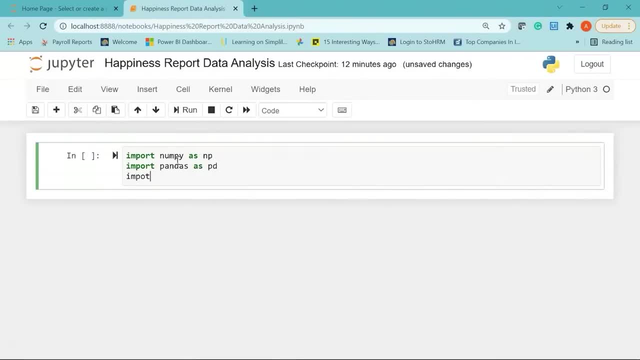 Then I will import two data visualization libraries, seaborn and matplotin. So I will say: import seaborn as sns and then import matplotlib dot pyplot, which is the module name, as plt And I will say % matplotlib inline. and Okay, Now let me just go ahead and run this. 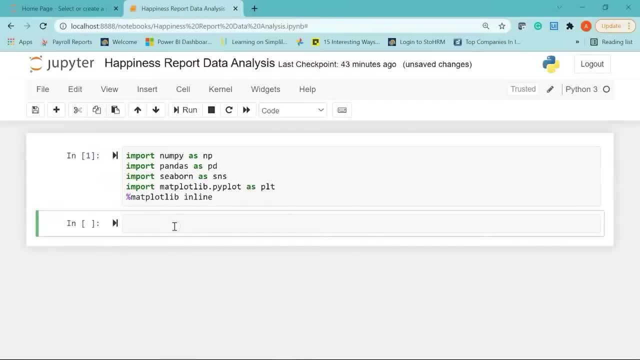 Alright. Well now let's set the parameters that control the general style of the plots. The style parameters control properties like the color of the background and whether a grid is enabled by default or not. So for that I will say sns dot set underscore style. 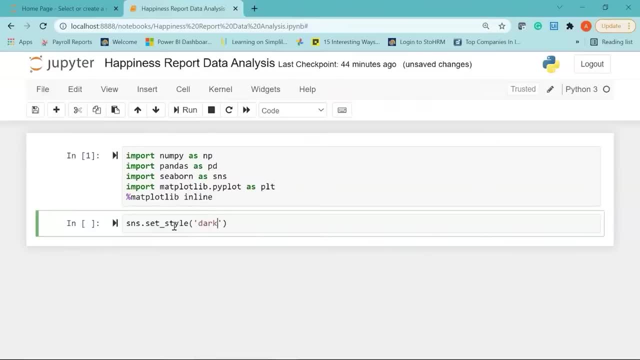 I will give it as dark grid. Next, I will say plt, dot, rc params, which stands for runtime configuration parameters. I am going to set my font size to, let's say, 15.. Then I will say plt- dot, rc params. Now I am going to 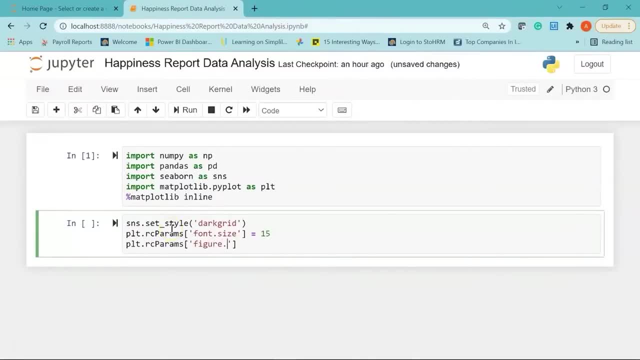 set the figure size, So I will say figure dot- fig size, Let's say 10,7. Next, I will just copy this, Paste it here. Now we are going to set the face color, So I will say figure dot- face color. 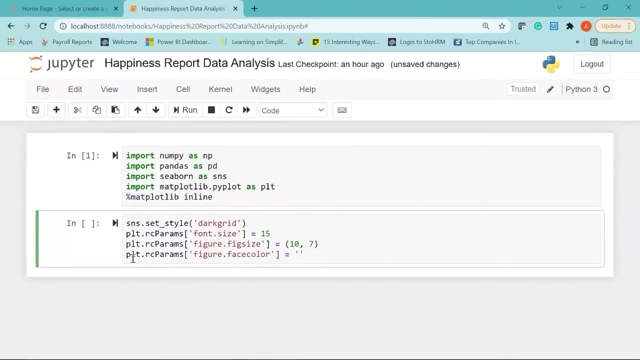 I want to set it to peach color, So I am going to pass in my RGB values for peach. I am going to set it in terms of hex code. So for peach, the value is ff, e, 5, b and 4.. Now let me run it. 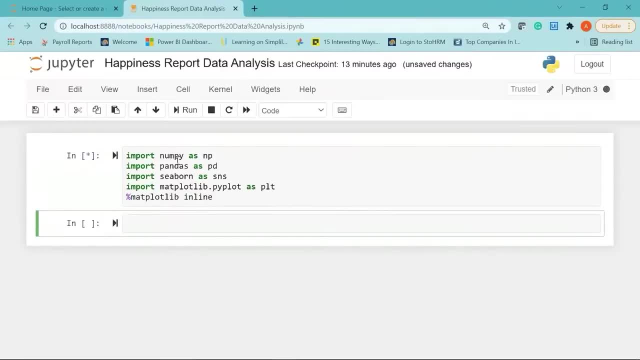 let me just go ahead and run this, alright. well, now let's set the parameters that control the general style of the plots. the style parameters control properties like the color of the background and whether a grid is enabled by default or not. so for that i will say sns. 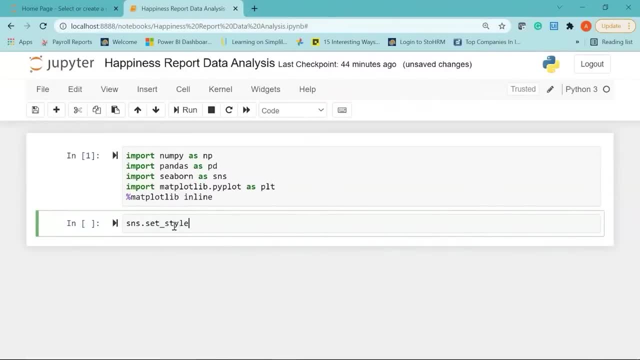 dot set under score style, i will give it as dark grid. next i will say plt, dot, rc params, which stands for runtime configuration parameters. i am going to set my font size to, let's say, 15. then i will say plt, dot, rc, params. now i am going to 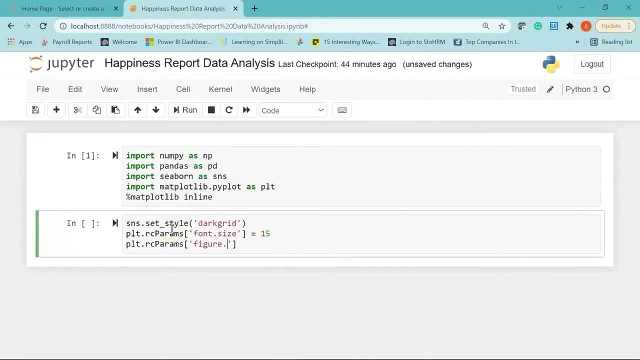 set the figure size, so i will say figure dot fig size. let's say 10 comma 7. next, just copy this, paste it here now we are going to set the face color, so i will say figure dot face color. i want to set it to peach color, so i am going to. 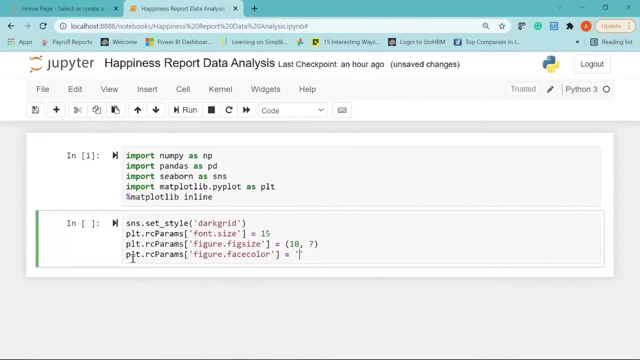 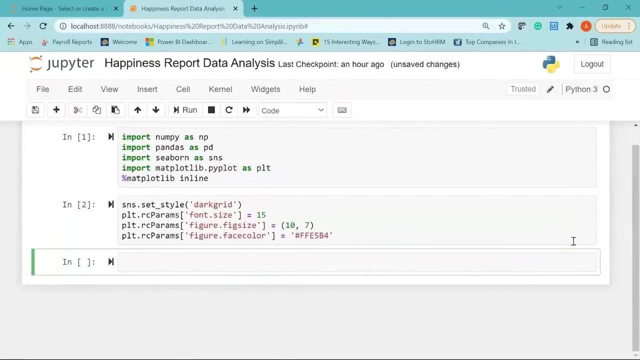 pass in my rgb values for peach. i am going to set it in terms of hex code. so for peach the value is ff, e, 5, b and 4. now let me run it. ok, now it's time to load our data set. so for that i will create a variable called data. 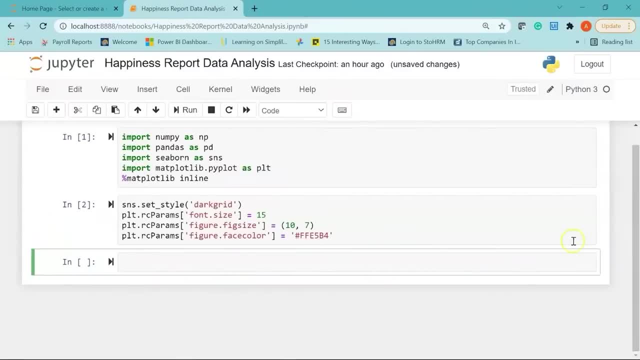 Ok, Now it's time to load our data set. So for that I will create a variable called data And I will use the pandas library, followed by the read underscore csv function, because our data set that we saw is a csv data set, which is this one. 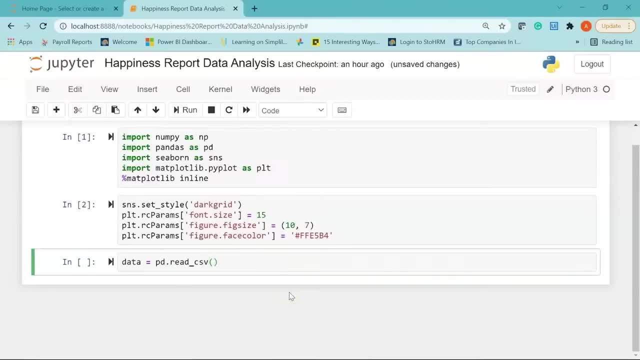 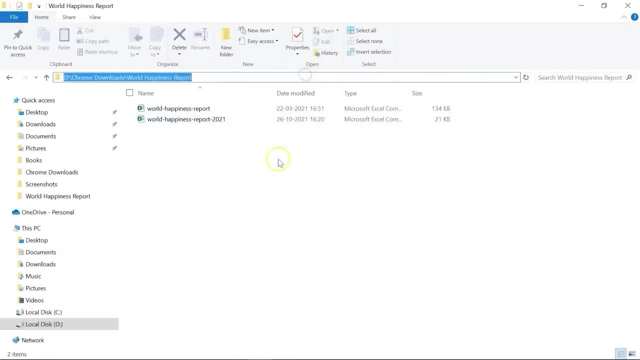 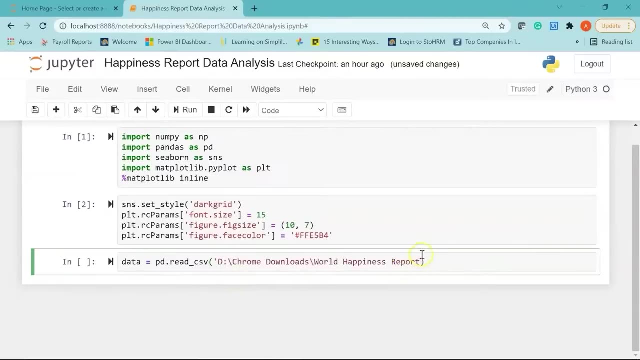 Now, inside the parenthesis, I will pass in the location of my data file. So I have my data here: World happiness report 2021.. I will just copy this location and will paste it here And make sure the location is within quotes And you need to change it to. 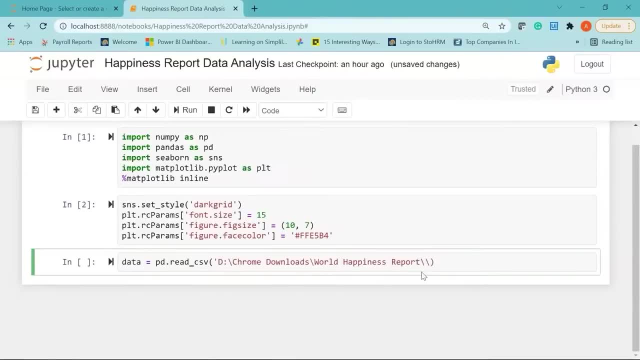 either forward slash or double backslash. So here I am using double backslash, So let me just include one more backslash And then I am going to pass in the file name, which is world hyphen, happiness, hyphen report, hyphen 2021. 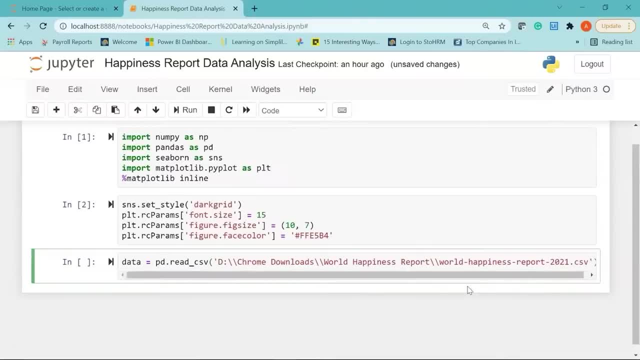 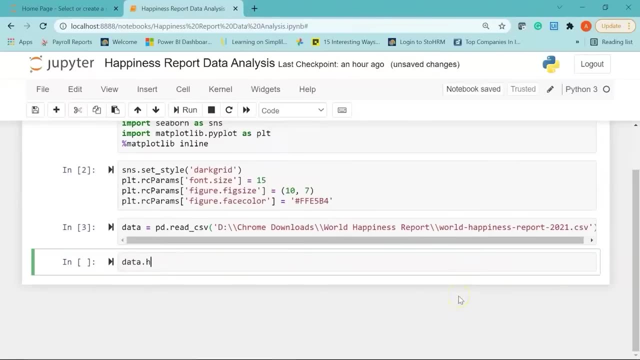 dot csv, which is the extension of the file. Now let me run it. Alright, Now to display the first five rows of information, you can use the head function. So I am writing data, which is my variable that holds the data frame. So data dot head. 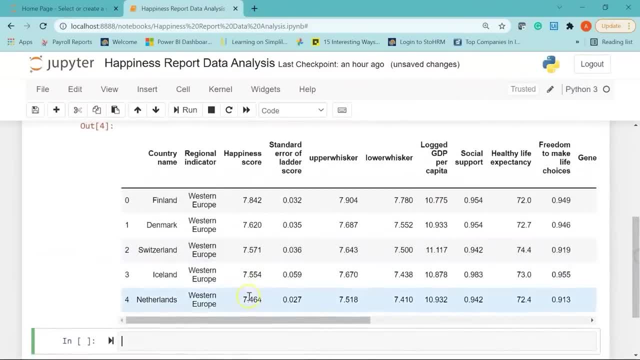 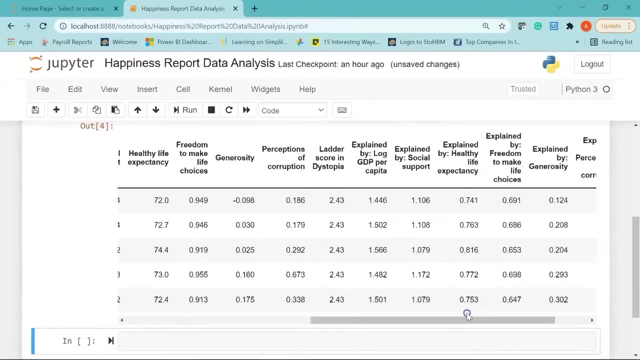 there you go. You can see here we have printed the first five rows from the data set. You have the country name, regional indicator, happiness score. Then we have information about the GDP, life expectancy, generosity. Then we have corruption data. 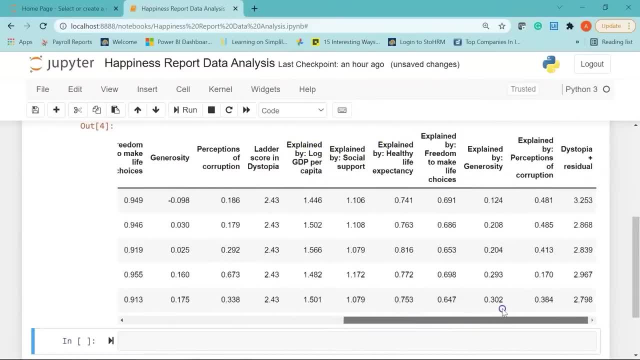 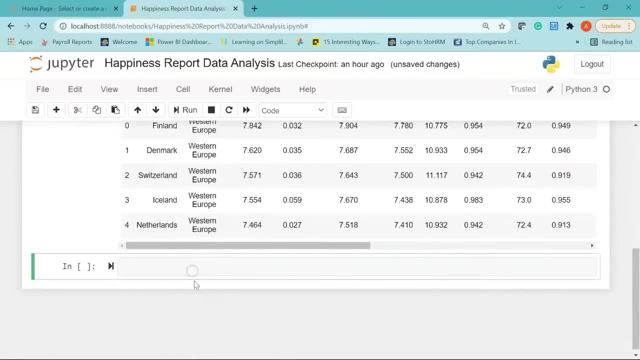 And these are some of the columns that we are not bothered about. So we are going to drop these columns from our analysis. Now, we are going to do that, So I will create a variable called data columns which are of our interest. So I am. 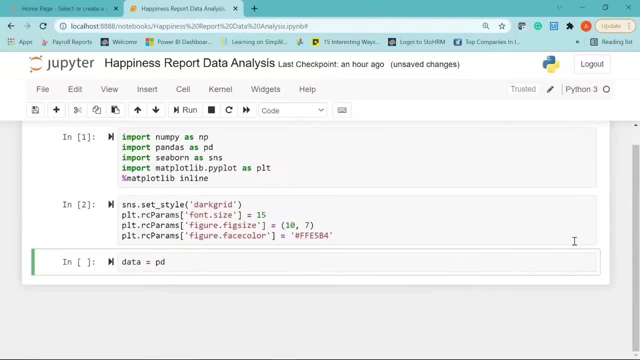 and i will use the pandas library, followed by the read underscore csv function, because our data set that we saw is a csv data set, which is this one. now, inside the parenthesis, i will pass in the location of my data file, so i have my data here. world happiness report 2021. 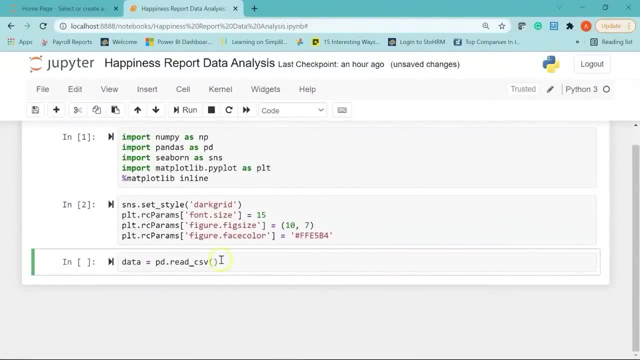 i will just copy this location and will paste it here and make sure the location is within quotes and you need to change it to either forward slash or double backslash. so here i am using double backslash, so let me just include one more backslash and then i am. 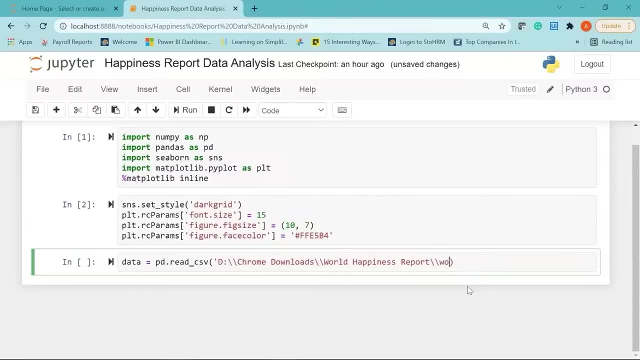 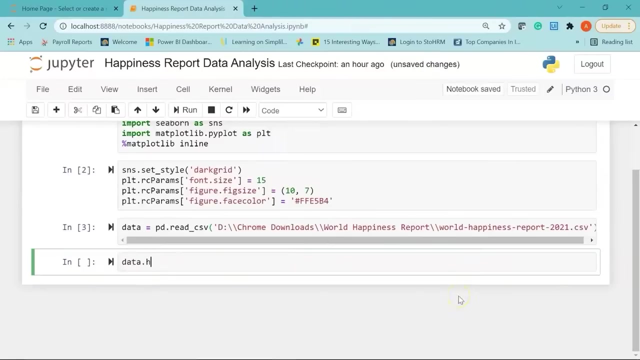 going to pass in the file name, which is world hyphen- happiness hyphen report- hyphen 2021 dot csv, which is the extension of the file. now let me run it alright. now to display the first five rows of information, you can use the head function. 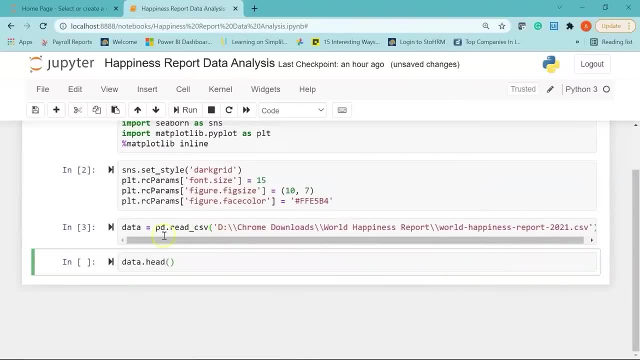 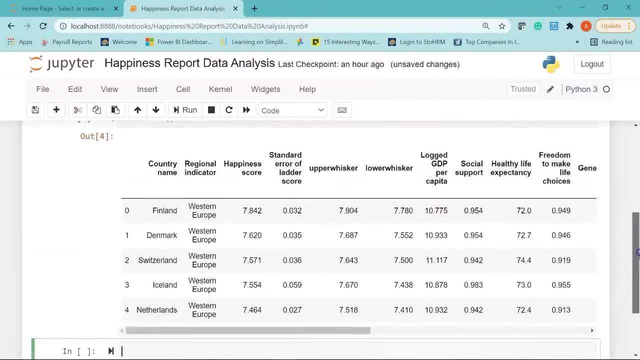 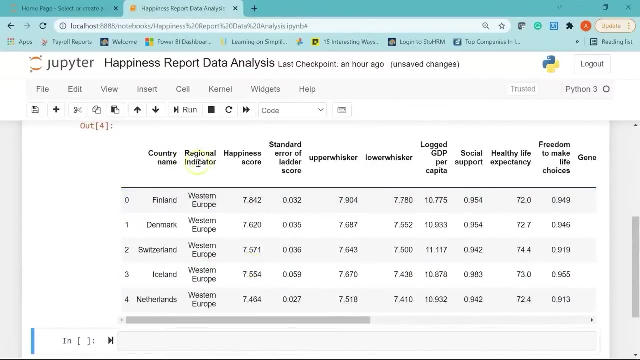 so i am writing data, which is my variable that holds the data frame. so data dot head. there you go. you can see here we have printed the first five rows from the data set. you have the country name, regional indicator, happiness score, then we have information about the gdp. 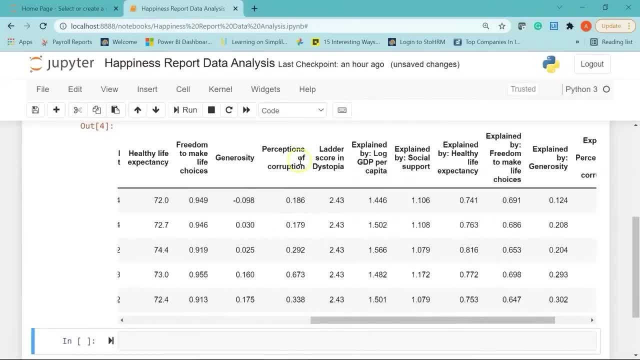 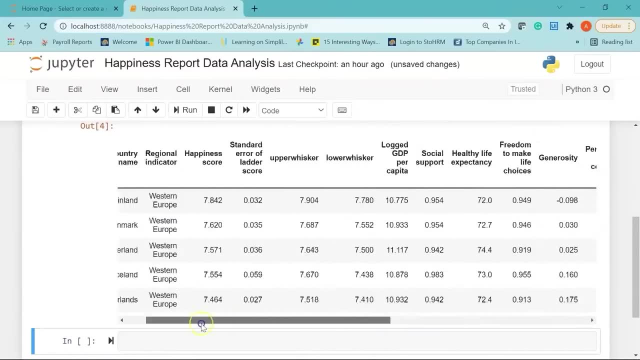 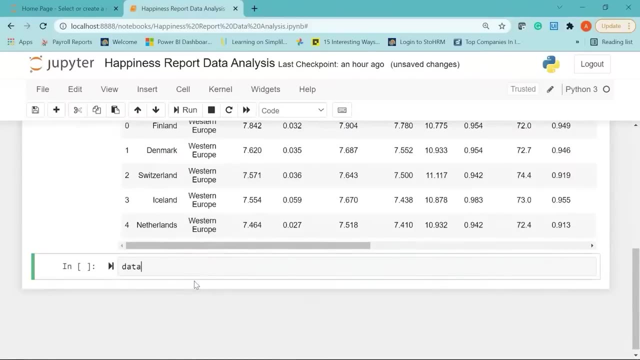 life expectancy, generosity. then we have corruption data, and these are some of the columns that we are not bothered about, so we are going to drop these columns from our analysis now. we are going to do that, so i will create a variable called data columns which are of our interest. 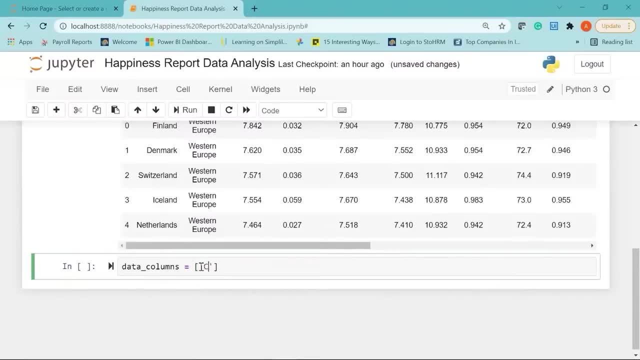 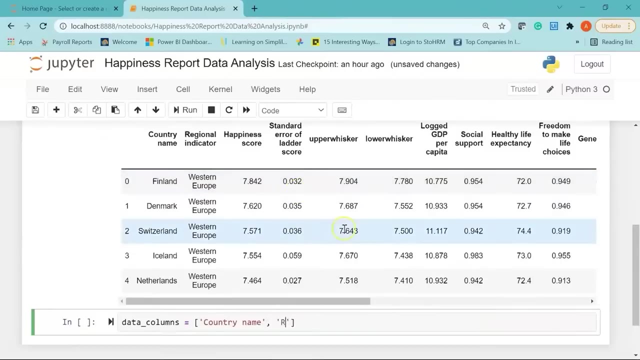 so i am going to take only specific columns. i need the country name, so i have taken country name. make sure the column names are within single quotes. so i have my country name. next i want the second column, which is regional indicator. give a comma. we also need the. 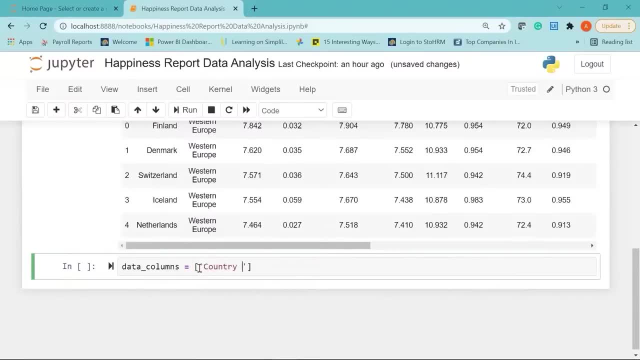 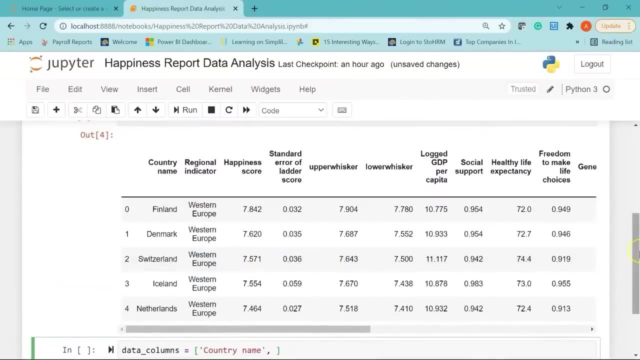 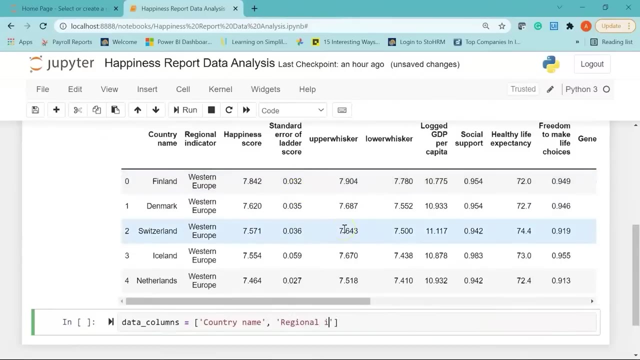 going to take only specific columns. I need the country name. So I have taken country name. Make sure the column names are within single quotes. So I have my country name. Next I want the second column, which is regional indicator. You give a comma. 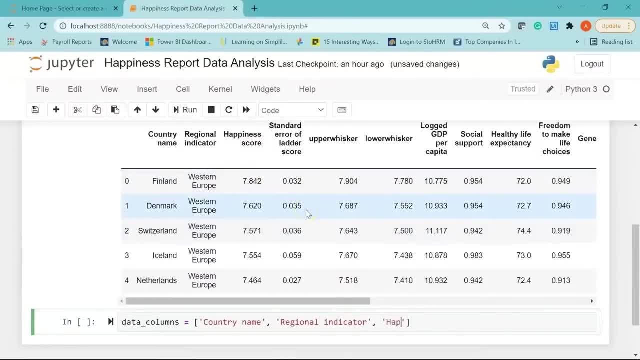 We also need the happiness score. Next, I need the logged GDP per capita data. So I will take that column. I will say: logged GDP per capita, Give a comma. My next column would be social support. Give a comma here. My next, 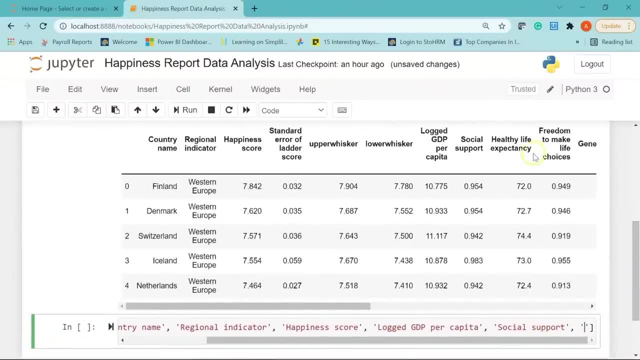 column would be health, life expectancy. So I will write health, life expectancy. Let's give another comma And we will take the next column as well, which is freedom to make life choices. So I will write that column name: Freedom to make life choices. 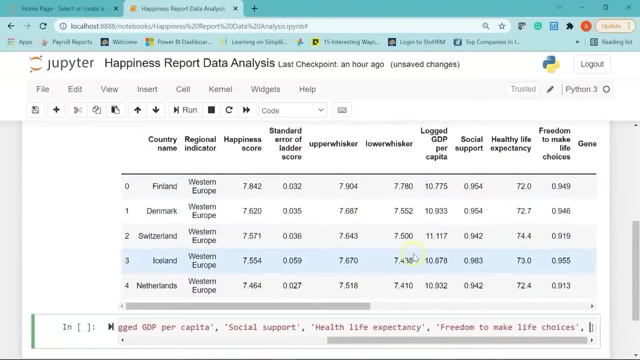 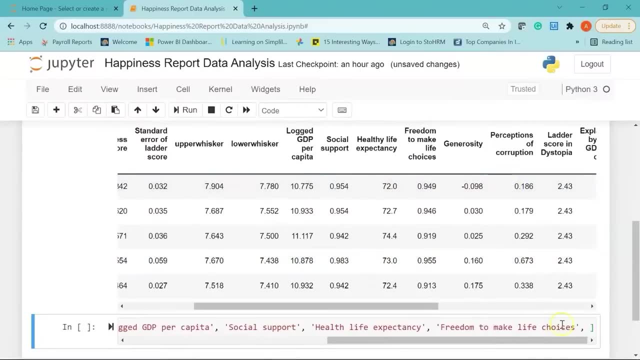 And finally, we will take the next two columns, that is, generosity and perceptions of corruption. So, within single quotes, I will say generosity, give a comma, and we are going to include the final column which is of our interest, that is, perceptions of corruption. Let me have a recheck. 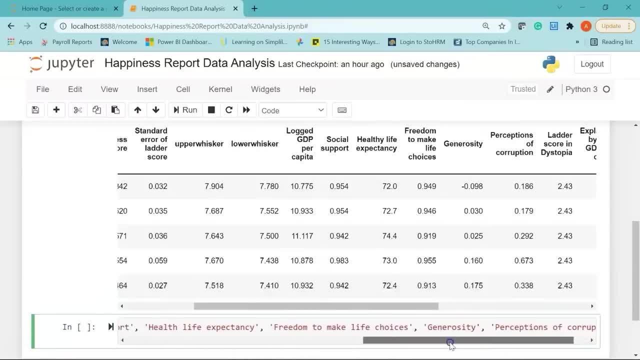 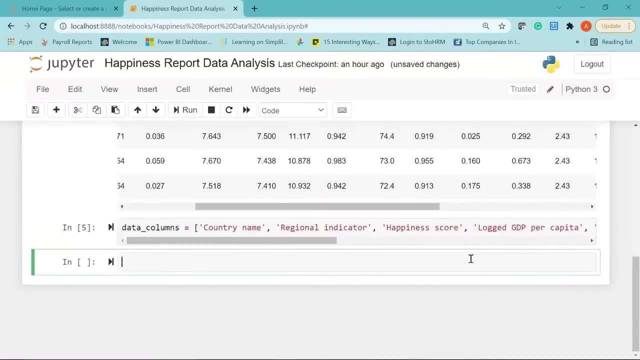 to ensure that I have put the column names correctly, Otherwise it will throw an error. Now let me go ahead and run this cell. I will hit shift, enter Alright. So we have successfully taken the columns that we will be using for an analysis Now. 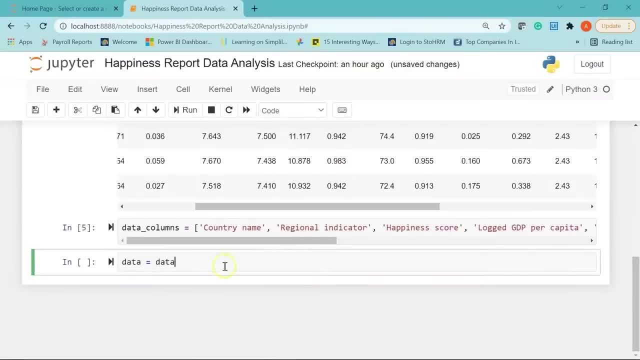 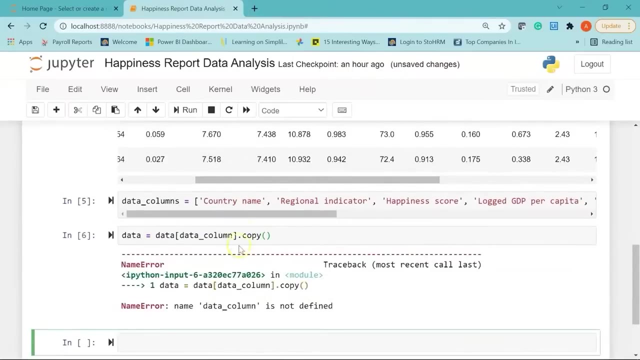 I am going to say data equal to data. I will pass in my new variable, that is data underscore columns, and I am going to copy all the data. So I will say dot copy. Let's run it. Okay, this should be data underscore columns. 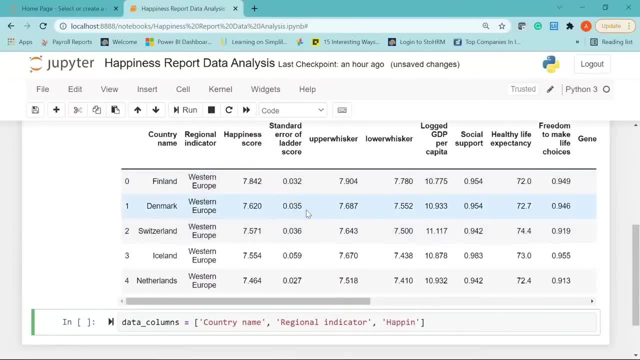 happiness score. next, i need the logged gdp per capita data. so i will take that column. i will say: logged gdp per capita, give a comma. my next column would be social support- give a comma here. my next column would be health- life expectancy. so i will write. 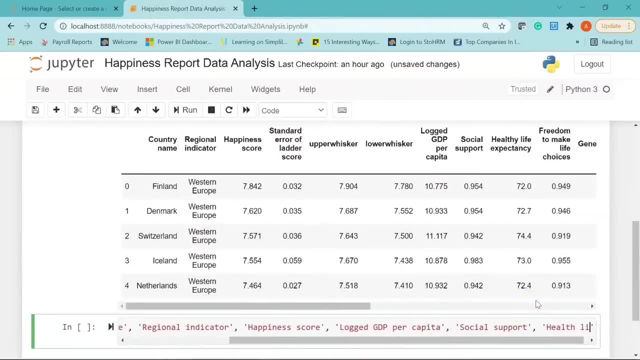 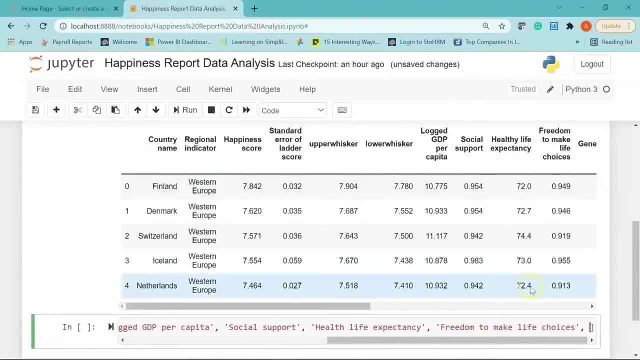 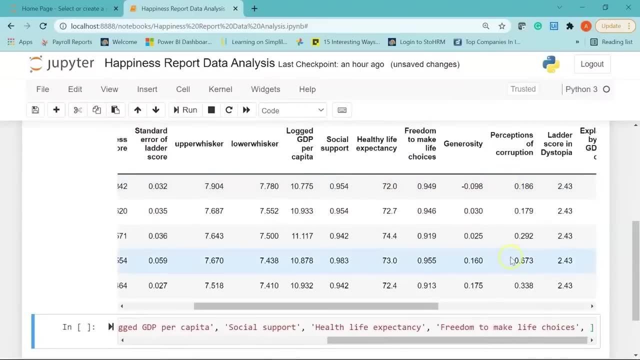 freedom to make life choices. and finally, we will take the next two columns, that is, generosity and perceptions of corruption. so within single quotes, i will say generosity, give a comma and we are going to include the final column which is of our interest, that is, perceptions of corruption. 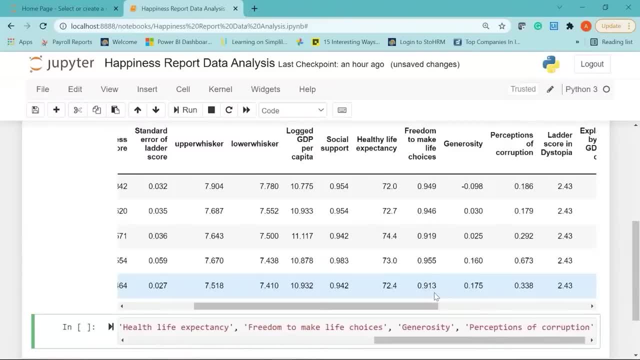 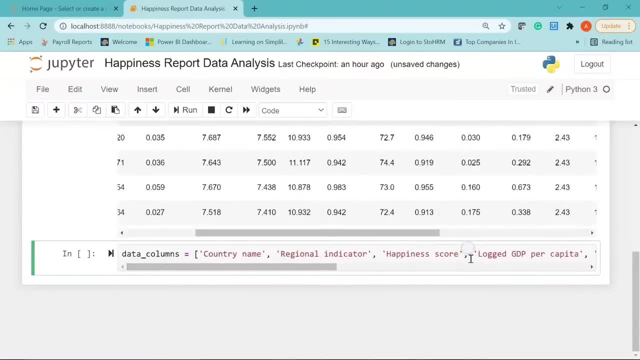 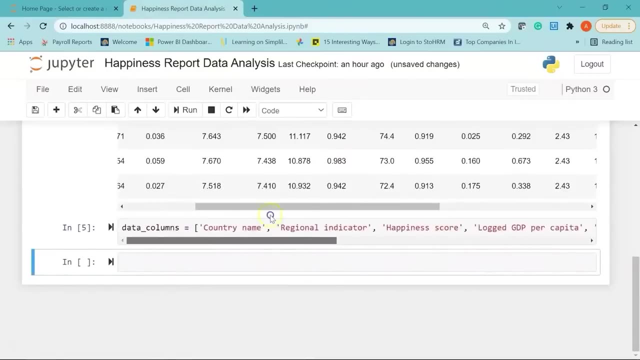 let me have a recheck to ensure that i have put the column names correctly, otherwise it will throw an error. now let me go ahead and run this cell. i will hit shift, enter. alright, so we have successfully taken the columns that we will be using for an analysis now. 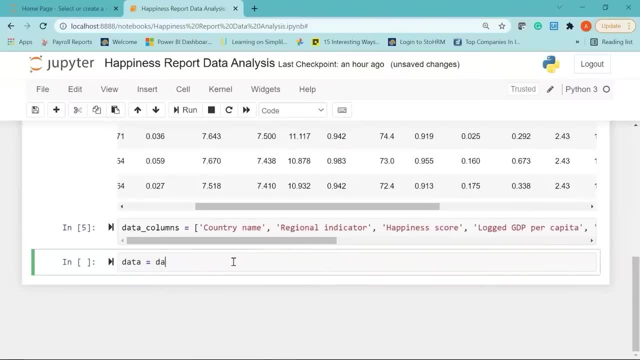 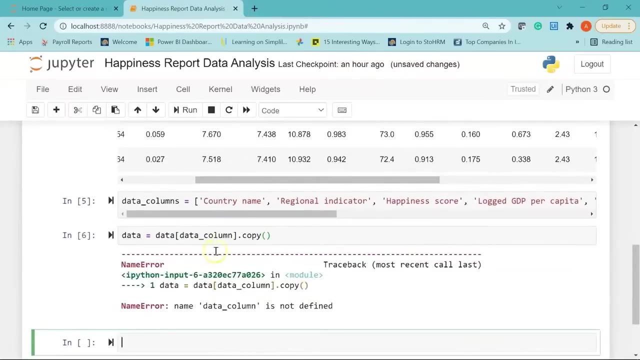 i am going to say data equal to data. i will pass in my new variable, that is data underscore columns, and i am going to copy all the data. so i will say dot, copy. let's run it. ok, this should be data underscore columns. alright, now let's rename all these. 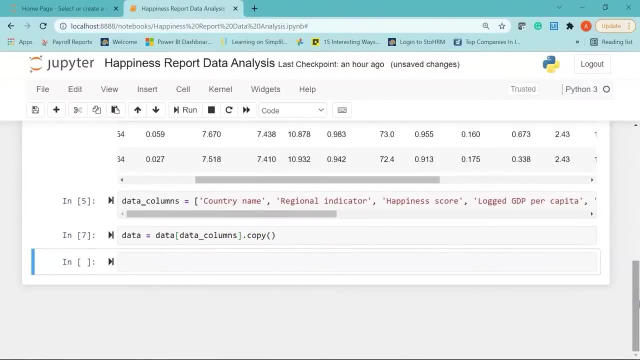 Alright, Now let's rename all these columns. We will make it more simpler and easy to understand. So I will say: let's say, my new variable is happy. underscore dear, which stands for data frame equal to. I will say data dot. we will use the rename function. 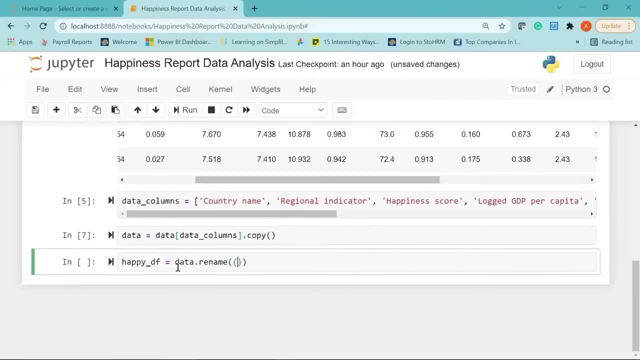 and using a dictionary, we will rename our columns. So I have used a curly bracket. I am going to pass in my first column, which is country name. I will just paste it here. Then I am going to give a colon and again within single. 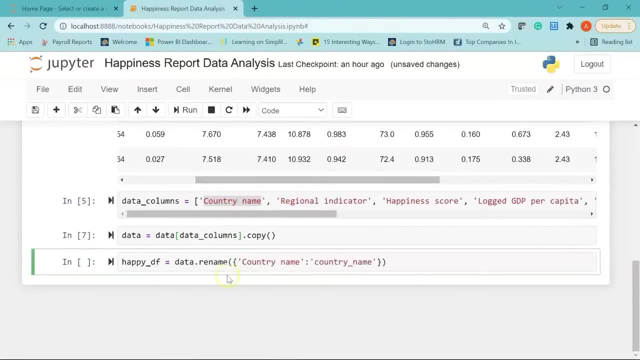 quotes. I will say country underscore name. So this is going to be my new column name. I will give a comma. We will take the next column, which is regional indicator. I will paste it here. Give a colon And the new column would be small. 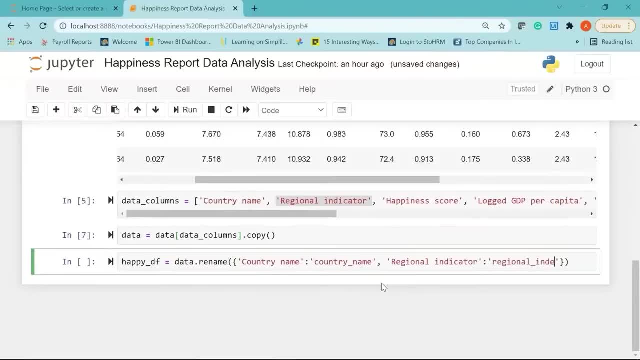 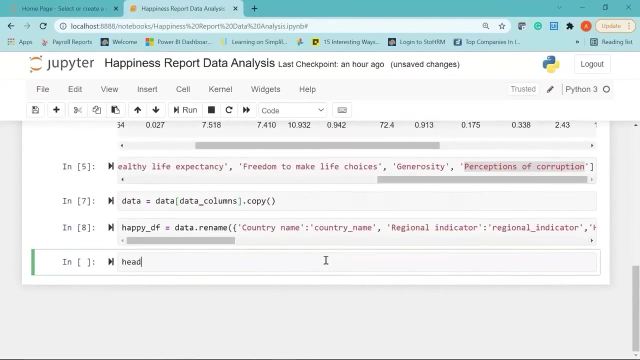 r- regional underscore indicator. Now, similarly, we will do this for all the remaining columns in the data set. Okay, Now I have renamed all my columns. You can see it here. Let's run it Now. we are going to display the head of the data set again. 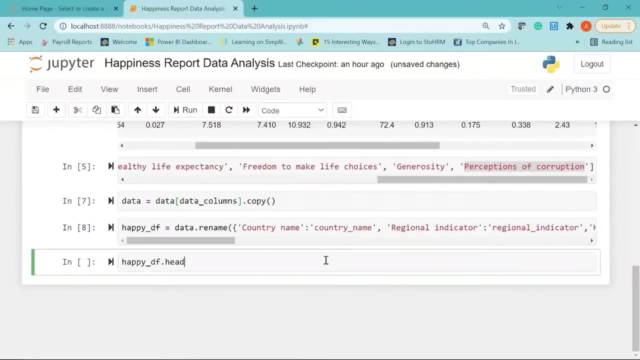 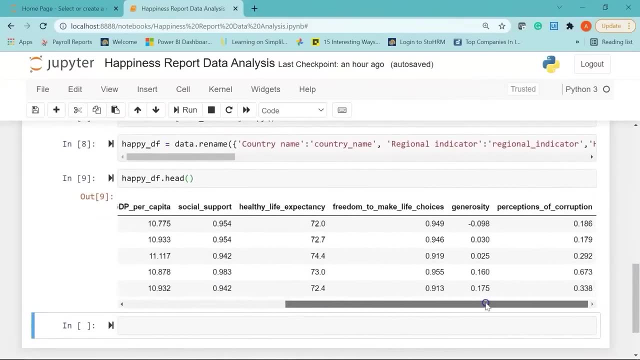 So I will say: happy, underscore: df dot head. There you go. So we have only those columns that are of our interest. So I have the country name, regional indicator, happiness score, GDP, social support, life expectancy, freedom to make life choices. 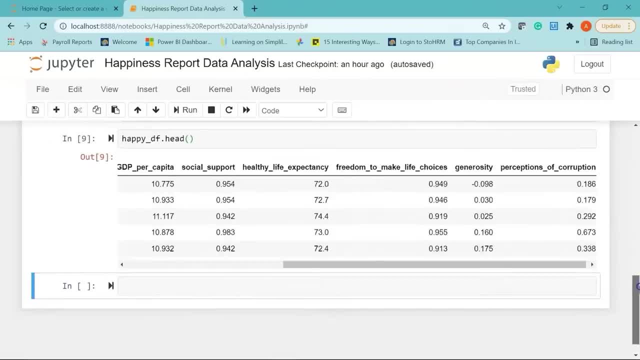 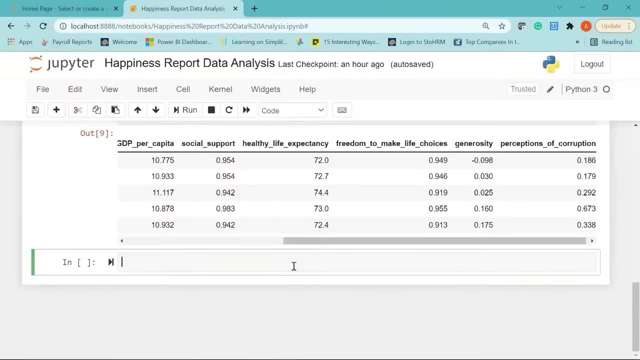 Then I have generosity and perceptions of corruption. Cool. Now we are going to check whether any of the columns have any null values. So for that I will say happy. underscore df dot. I am going to use the is null function. I will give another dot and 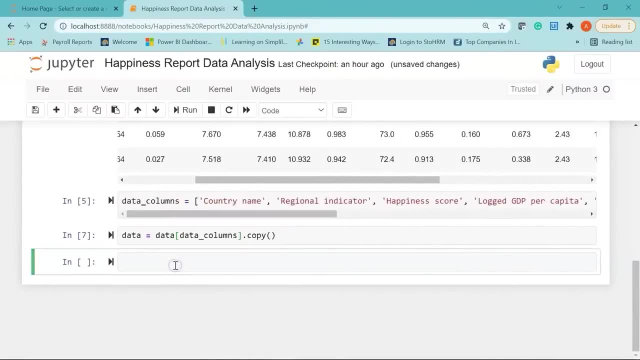 columns. we will make it more simpler and easy to understand. so i will say: let's say, my new variable is happy. underscore dear, which stands for data frame equal to, i will say, data dot. we will use the rename function and, using a dictionary, we will rename our columns. so i have: 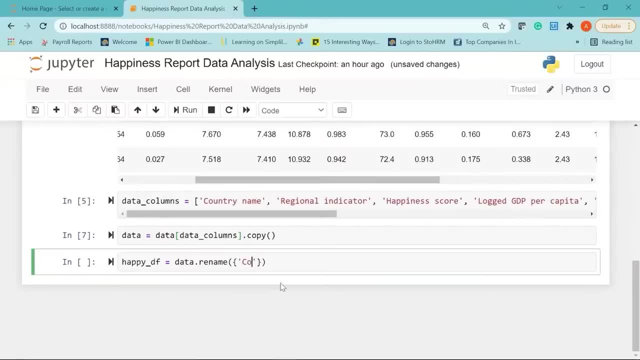 used a curly bracket. i am going to pass in my first column, which is country name. i will just paste it here. then i am going to give a colon and again, within single quotes, i will say country underscore name. so this is going to be my new column name. 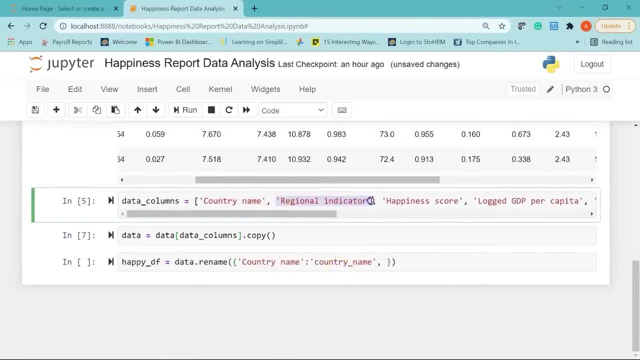 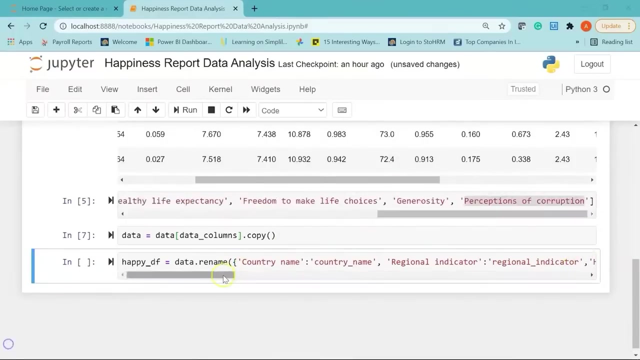 i will give a comma. we will take the next column, which is regional indicator. i will paste it here. give a colon and the new column would be small r, regional underscore indicator. now, similarly, we will do this for all the remaining columns in the data set. ok, now i have renamed all my columns, you can. 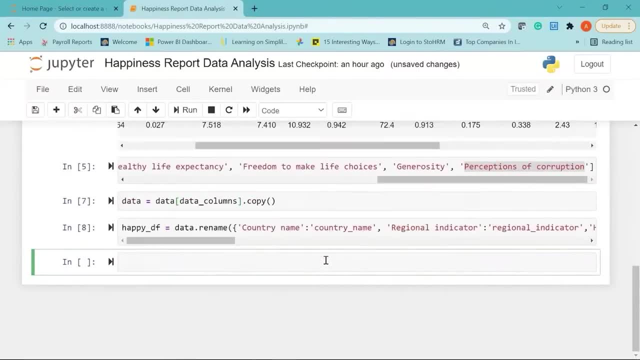 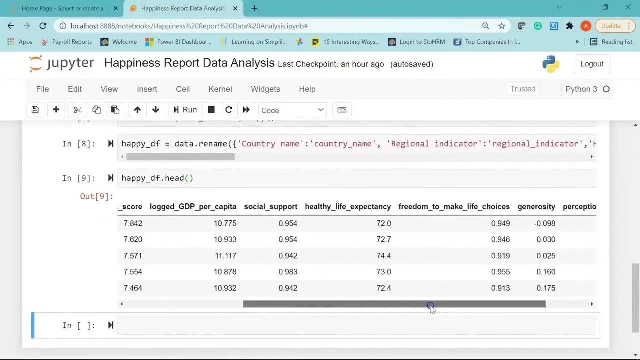 see it here? let's run it now. we are going to display the head of the data set again. so i will say happy, underscore: df, dot head. there you go. so we have only those columns that are of our interest. so i have the country name. regional indicator. 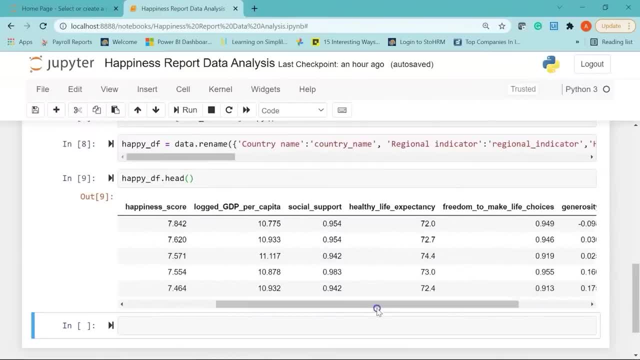 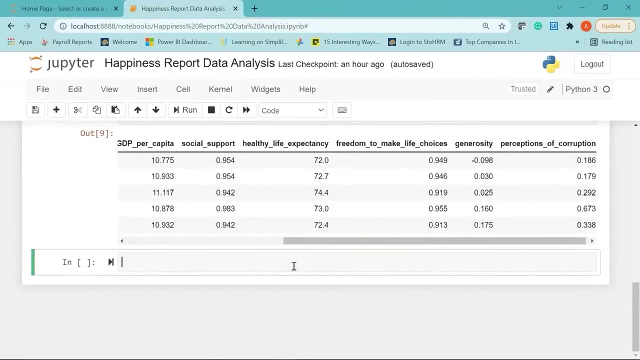 happiness score, gdp, social support, life expectancy, freedom to make life choices. then i have generosity and perceptions of corruption. cool, now we are going to check whether any of the columns have any null values, so for that i will say happy. underscore df dot i am going to use 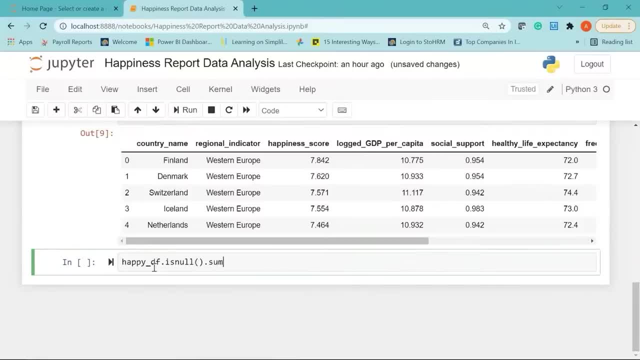 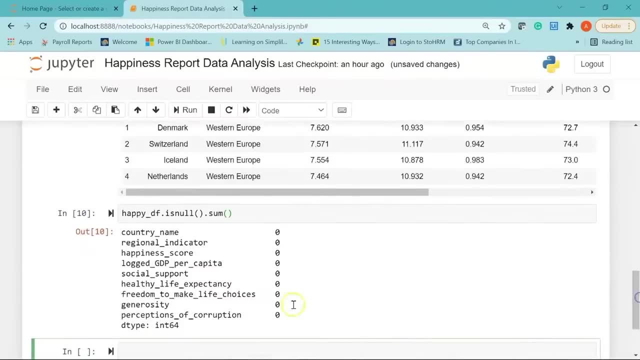 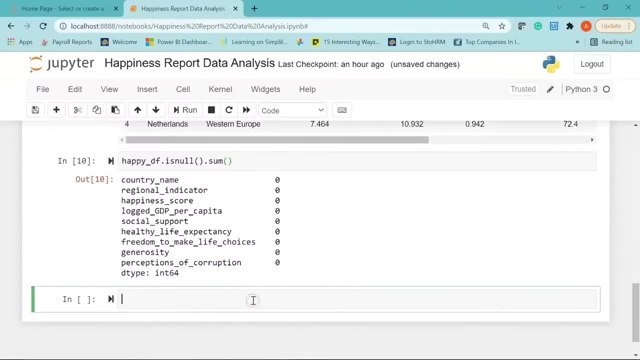 the is null function. i will give another dot and we are going to find the sum for each of the columns. you can see from the data, we do not have any null values in any of the columns in the data set. it is all zero. ok, now let's get started with our 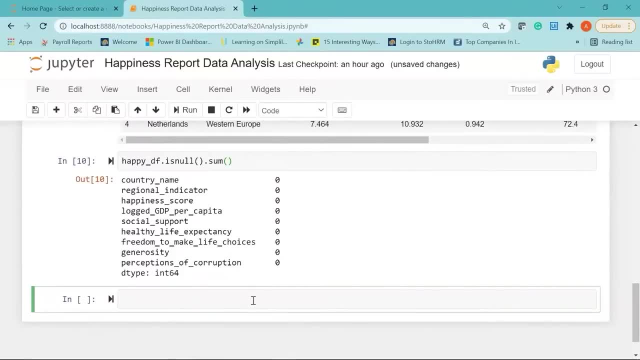 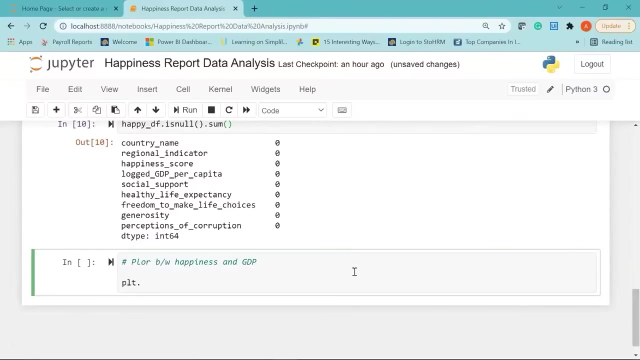 first visualization, that is, we will create a plot between happiness score and the gdp for different regions. so for that i will give a comment. as plot between happiness and gdp i will just scroll down, cool. first i am going to set the rc parameters, so i will say plt dot. 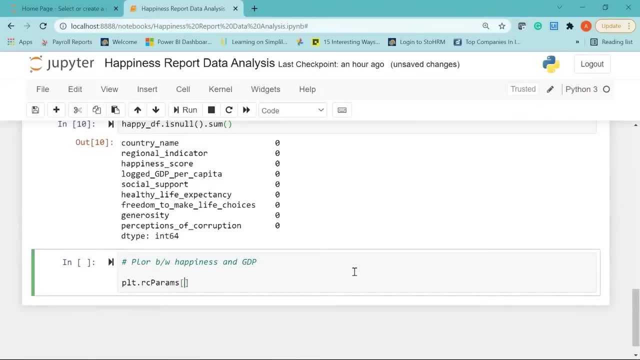 rc params within square brackets. i am going to give my figure size, so i will say figure dot fix size equal to. let's say my figure size is 15 comma 7. i will set the title, that is dot title of my plot, to, let's say: 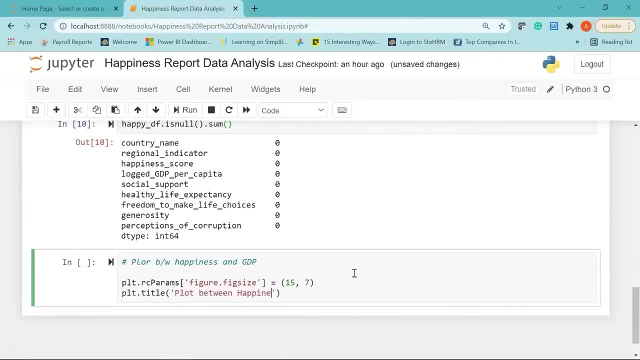 plot between happiness score and gdp. next, i am going to say sns dot. let's create a scatter plot. so i will say sns dot, scatter plot. i am going to define my x axis and the y axis for the plot. let's say: in the x axis we have 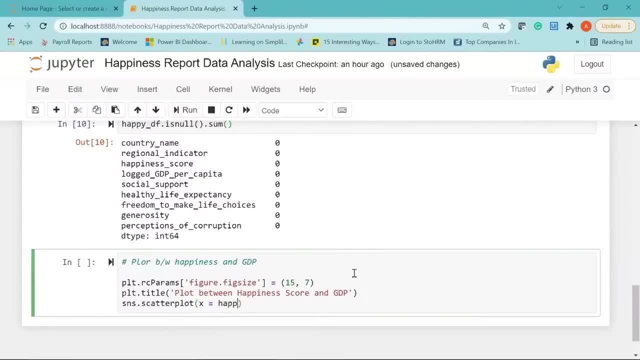 my data frame: happy underscore, df, dot. this should be an underscore. i will say column name as happiness underscore score. give a comma and in the y axis we will have my data frame name. that is: happy underscore, df, dot. we will have the gdp column, that is. 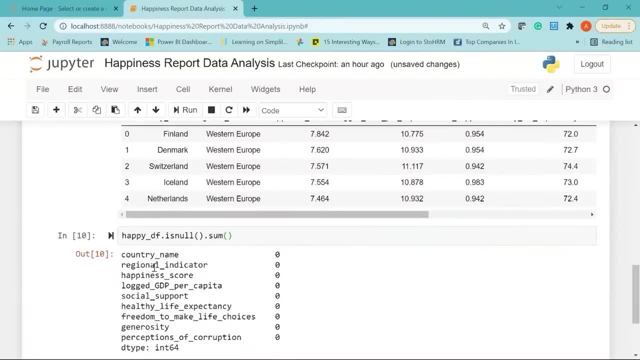 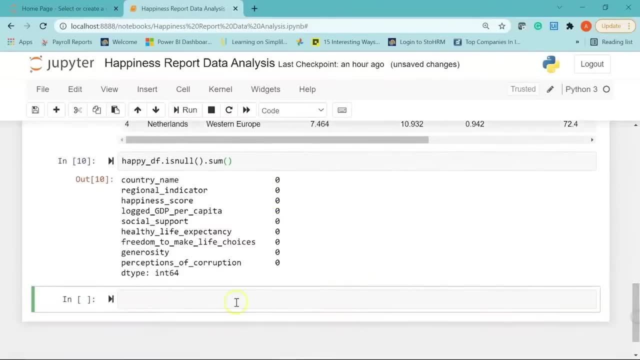 we are going to find the sum for each of the columns. You can see from the data, we do not have any null values in any of the columns in the data set It is all zero. Okay, Now let's get started with our first visualization, that is: 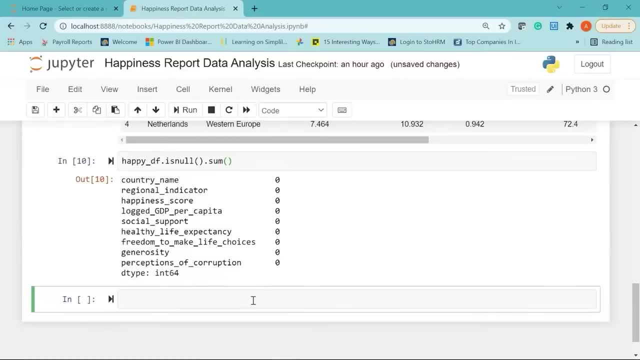 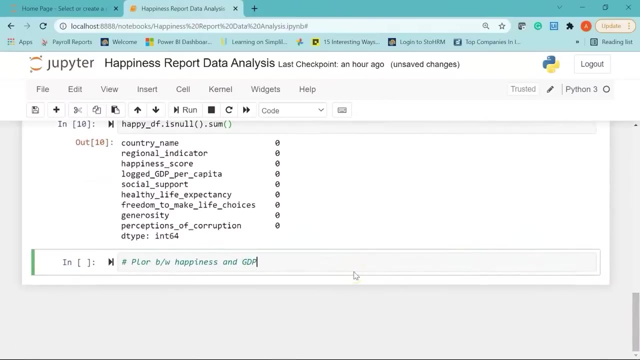 we will create a plot between happiness score and the GDP for different regions. So for that I will give a comment as plot between happiness and GDP, I will just scroll down Cool. First I am going to set the RC parameters, So I will say: 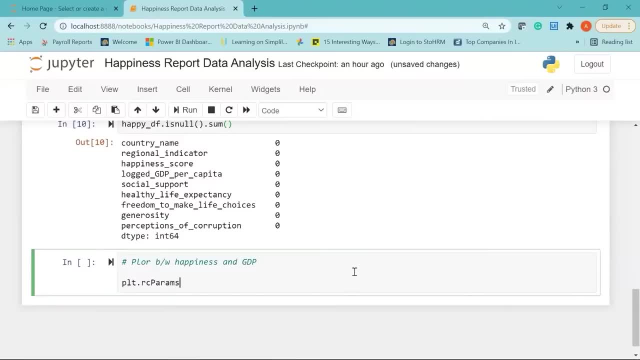 PLT dot. RC. params within square brackets. I am going to give my figure size, So I will say figure dot fixed size equal to, let's say, my figure size is 15 comma 7.. I will set the title, that is, PLT dot. 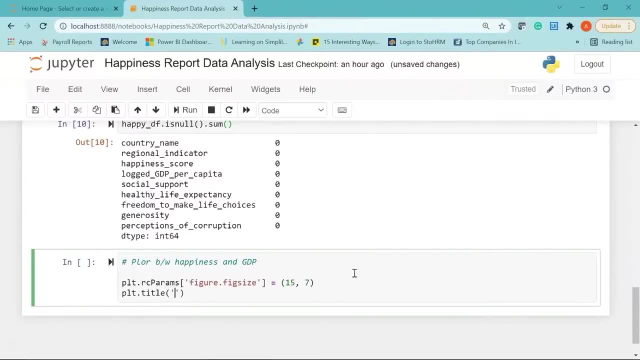 title of my plot to, let's say plot between happiness score and GDP. Next, I am going to say SNS dot, let's create a scatter plot. So I will say SNS dot, scatter plot. I am going to define my X axis and the Y axis for the plot. 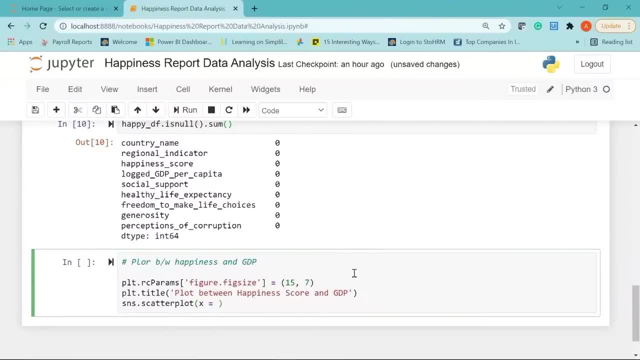 Let's say in the X axis we have my data frame happy underscore- DF dot. this should be an underscore. I will say column name as happiness underscore score. Let's give a comma. and in the Y axis we will have my data frame name. that is happy underscore DF dot. 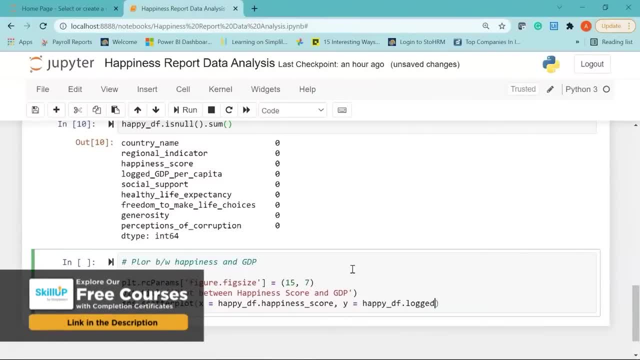 we will have the GDP column that is logged underscore GDP, underscore per, underscore capita. Let's give a comma and we will pass in hue. for the color, Let's say: for hue, I am going to use the regional column or the regional indicator column, so I will say: 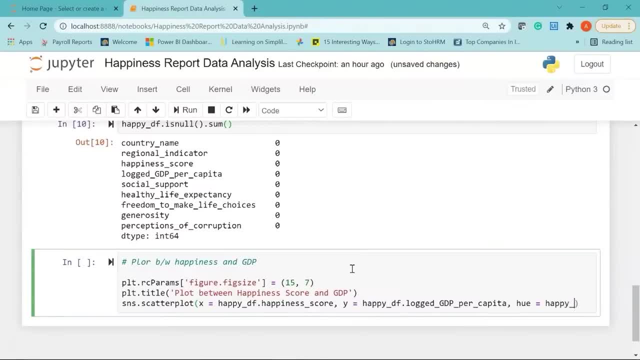 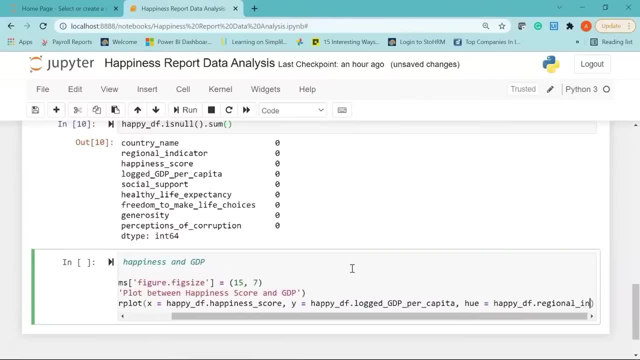 happy underscore: DF dot, regional underscore indicator. and then I am going to give the size of the dots, as let's say 200. then I will give a semicolon. come to the next line. I will say PLT- dot. let me just scroll down. now we are going to 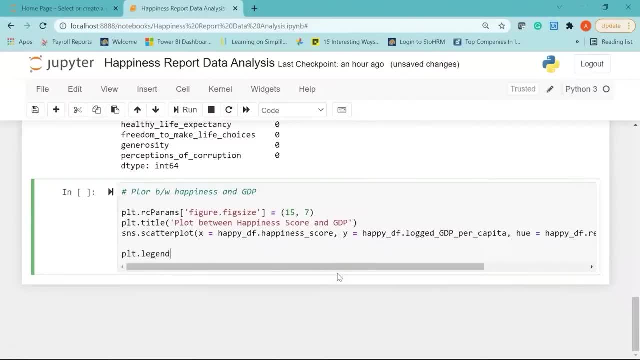 define the legend. so I will say PLT dot legend and in legend we will have the location. let's say I want to put the legend at upper left corner, so I will say loc, which is for location equal to upper left, give a comma and then say: 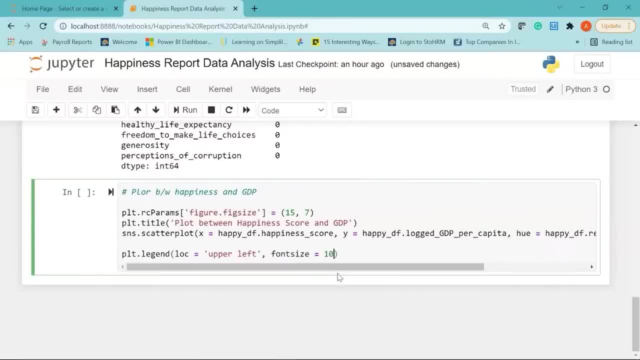 font size of my legend let's say be 10. make sure this is within quotes. then I am going to pass my x axis labels and the y axis labels. so I will say PLT dot x label. let's say the x label is happiness score and my y label is: 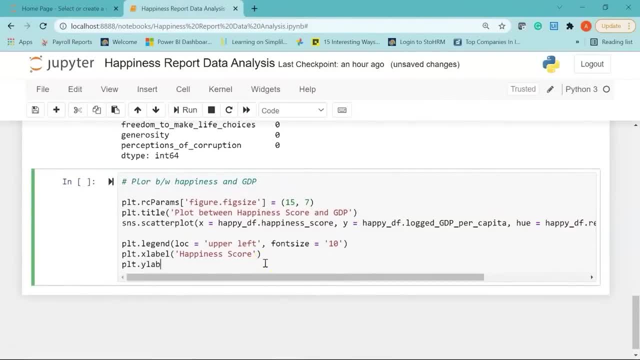 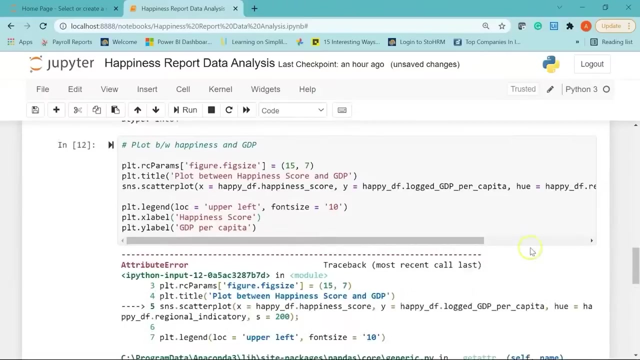 GDP per capita. so I will say PLT dot y label within single quotes, I will say GDP per capita. there is an error here. this should be plot, alright. so I have written my code to create a scatter plot. let's run it and see the result. there is some error here. 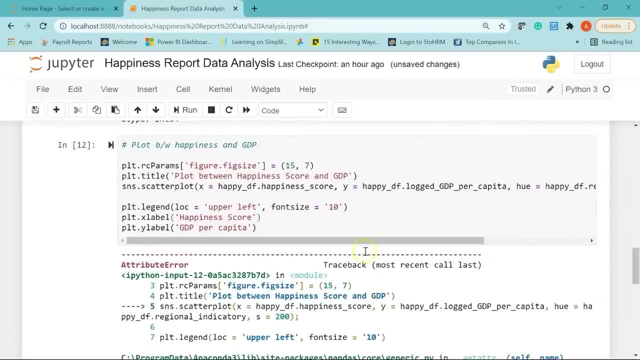 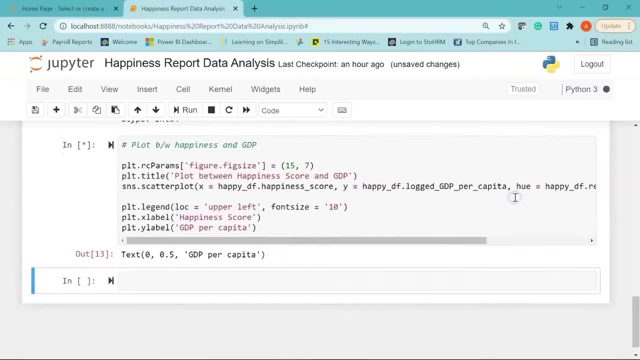 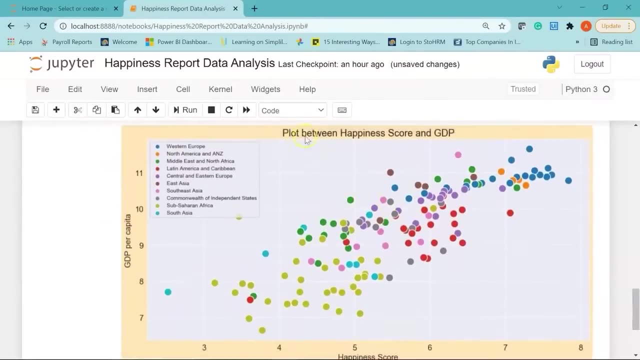 ok, this should be regional indicator and not indicator. there is a spelling mistake. let's run it again. alright, so here you can see we have a nice scatter plot. on the top you can see we have the title of the plot, that is, plot between happiness score and GDP. 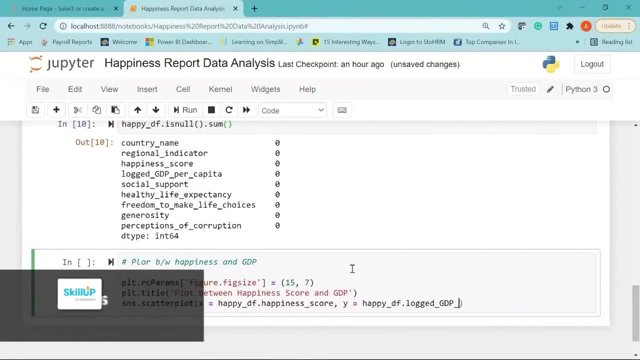 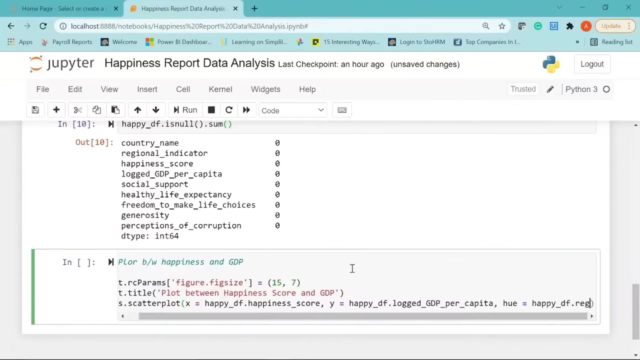 logged. underscore gdp, underscore per, underscore capita. let's give a comma and we will pass in hue for the color. let's say for hue, i am going to use the regional column or the regional indicator column, so i will say happy. underscore df dot. regional underscore indicator. 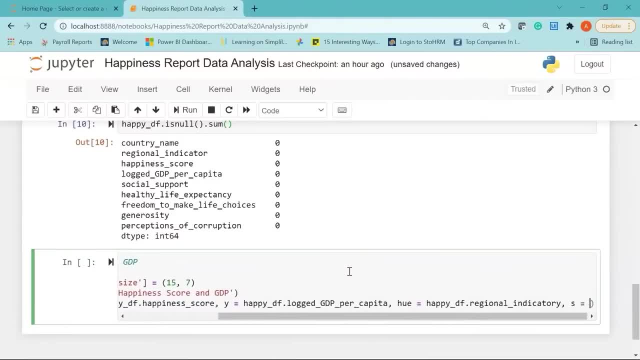 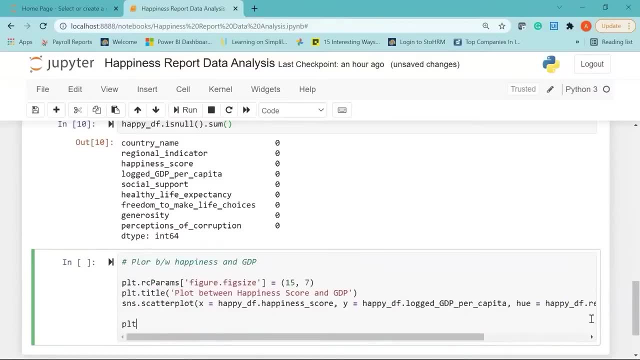 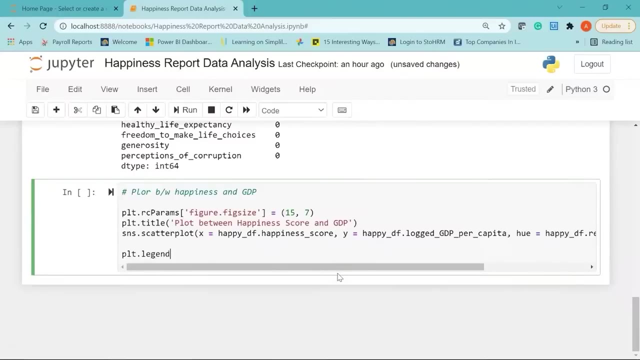 and then i am going to give the size of the dots, as let's say 200. then i will give a semicolon. come to the next line. i will say plt dot. let me just scroll down. now we are going to define the legend, so i will say plt dot. 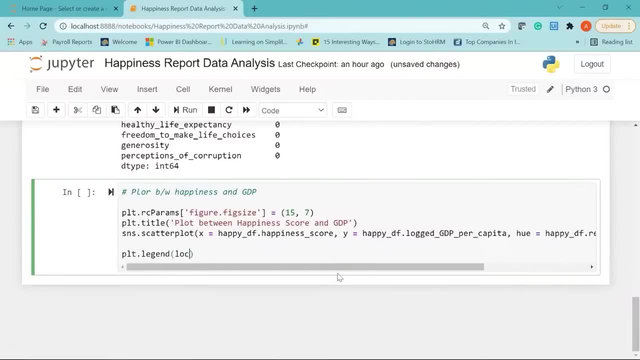 legend and in legend we will have the location. let's say i want to put the legend at upper left corner, so i will say loc, which is for location equal to upper left, give a comma and then say font size of my legend, let's say be 10 make. 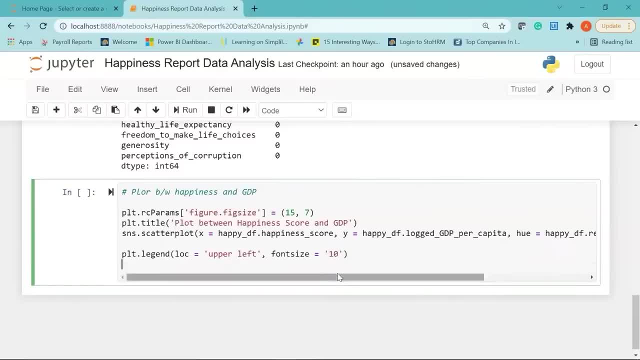 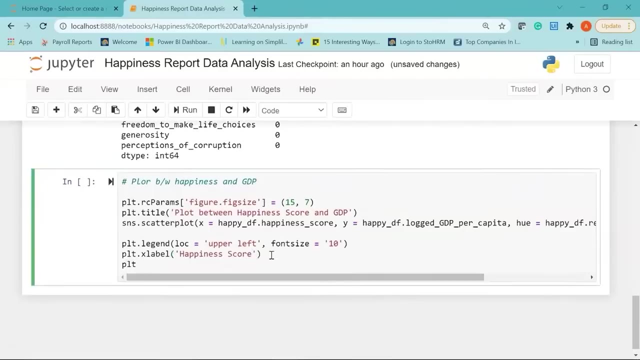 sure this is within quotes. then i am going to pass my x axis labels and the y axis labels. so i will say plt dot x label. let's say the x label is happiness score and my y label is gdp per capita. so i will say plt dot y. 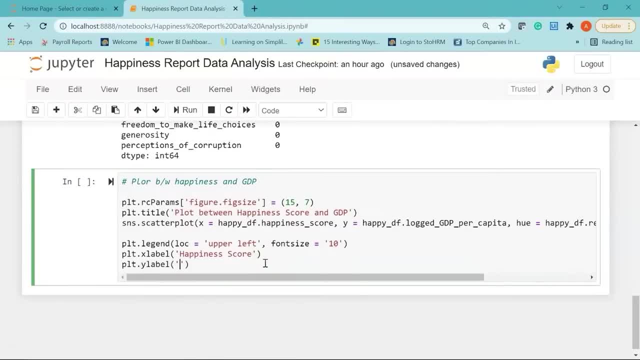 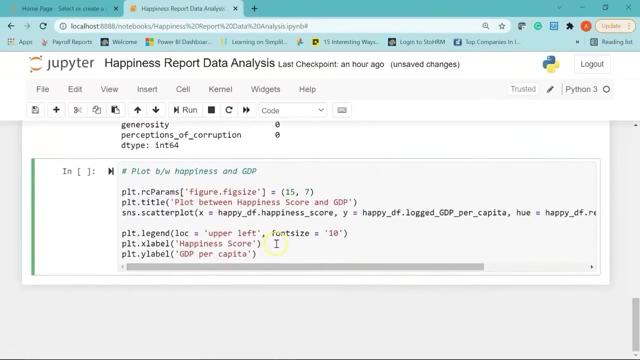 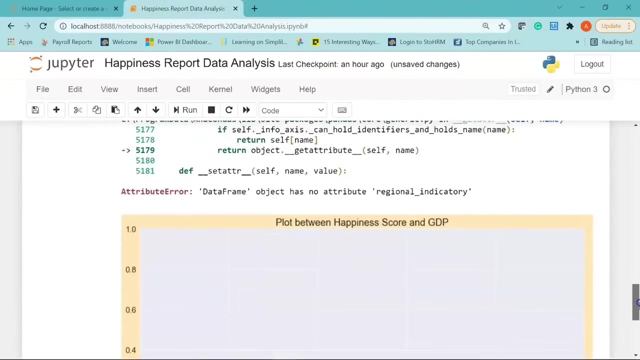 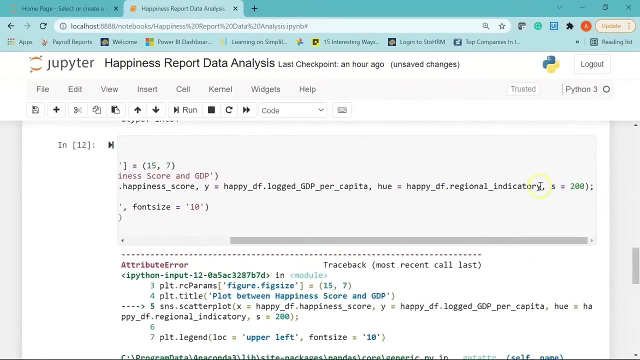 label. within single quotes, i will say gdp per capita. there is an error here. this should be plot. alright, so i have written my code to create a scatter plot. let's run it and see the result. there is some error here. ok, this should be regional indicator. 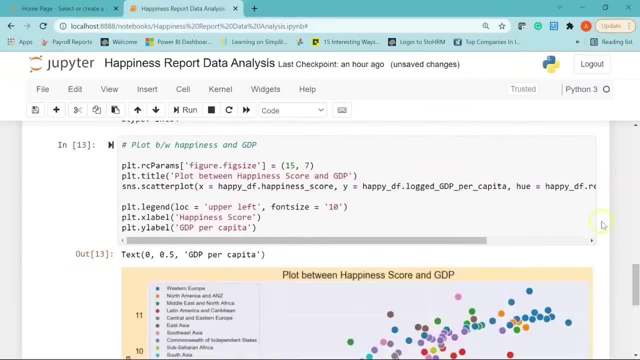 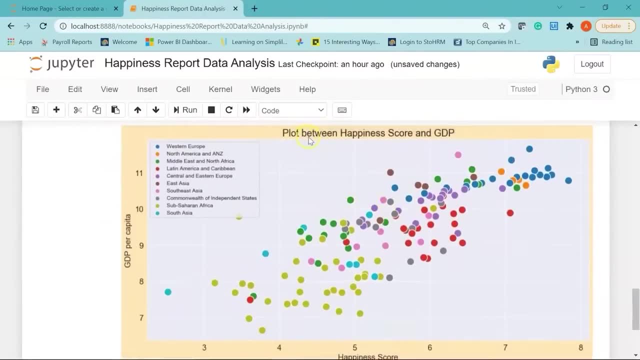 and not indicator. there is a spelling mistake. let's run it again. alright, so here you can see we have a nice scatter plot. on the top you can see we have the title of the plot, that is, plot between happiness score and gdp. on the x axis we have the happiness. 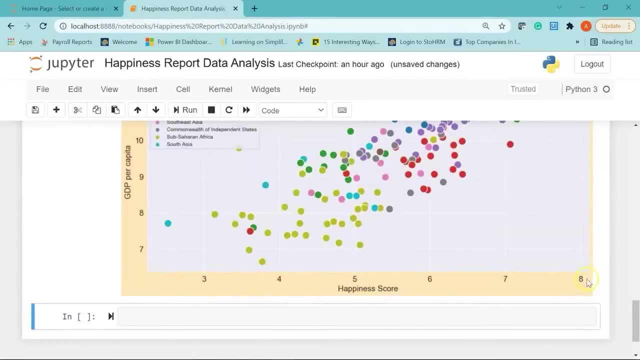 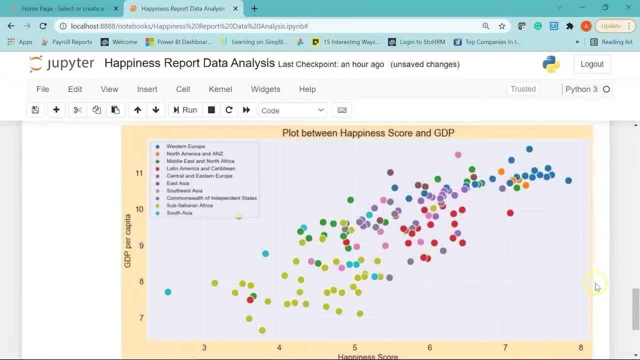 on the x axis we have the happiness score from 0 to 8 and above, and on the y axis you have the GDP per capita and if you see, here in this region we have countries from western europe which have the highest happiness score and the GDP. 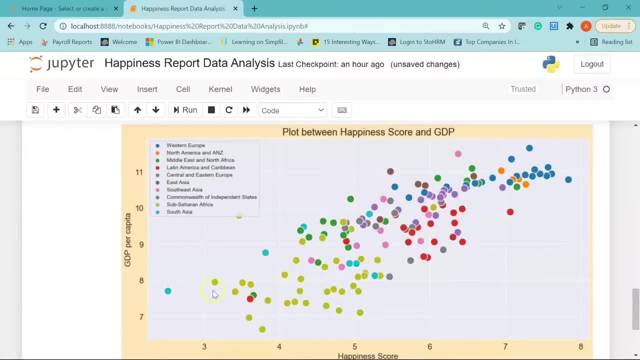 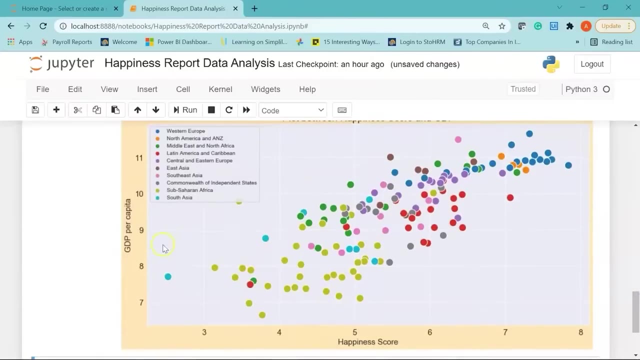 per capita is also the highest around this region. you can see here which is for green and in the legend you can see green is for sub saharan africa. so all these countries have low happiness score and even the GDP per capita is also low and if you see the 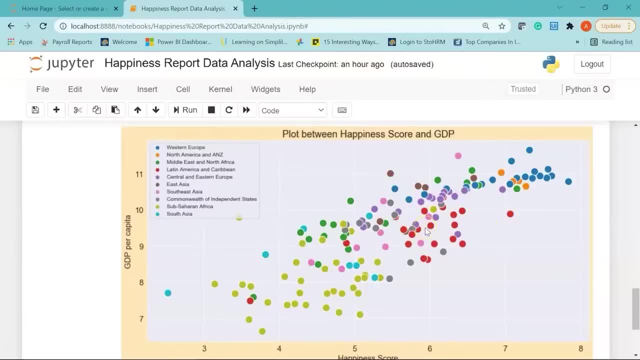 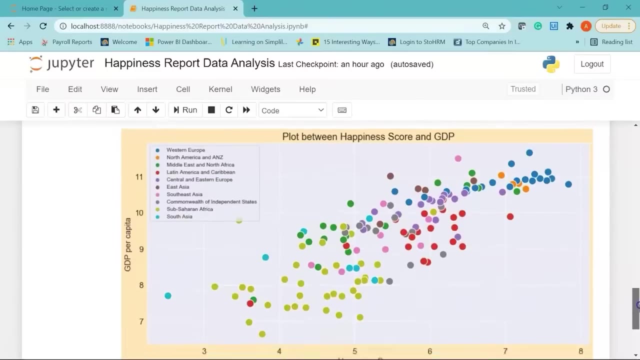 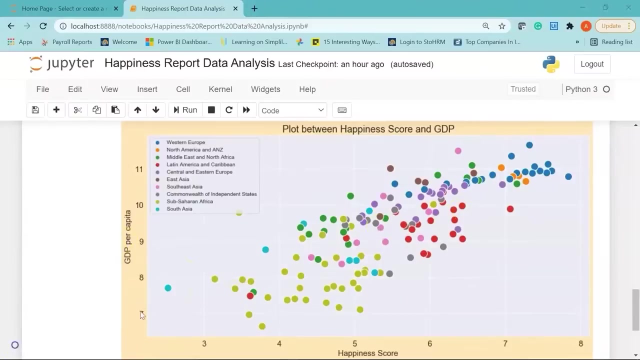 countries for Latin America and Caribbean. you see a lot of the values lie here, so they are all within the range of 5.5 to 7 in happiness score and even the GDP per capita is more than 9 for most of them. now, even the 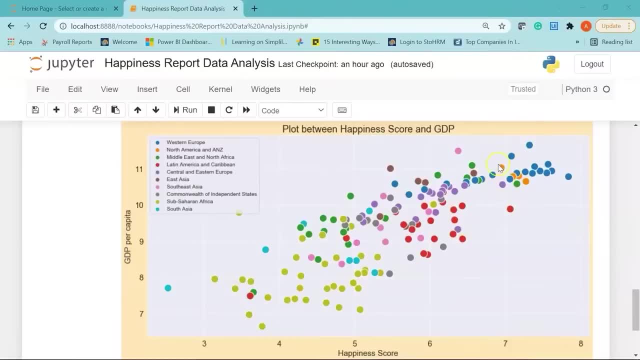 happiness score is high for the countries that lie in the North America and ANZ region, and even their GDP per capita is also the highest. I can name a few countries such as Australia, New Zealand. we have Canada and United States of America, which belong to the North America and ANZ. 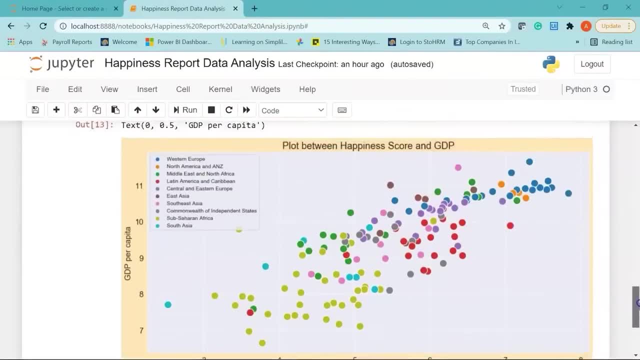 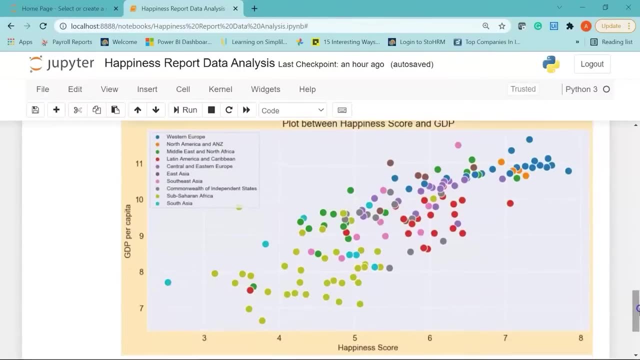 region cool. now there is one country which you see here. this seems to be like an outlier, which means that this is the country which has the lowest happiness score and even the GDP per capita is also low. but it is not the lowest because, you can see here there are a few. 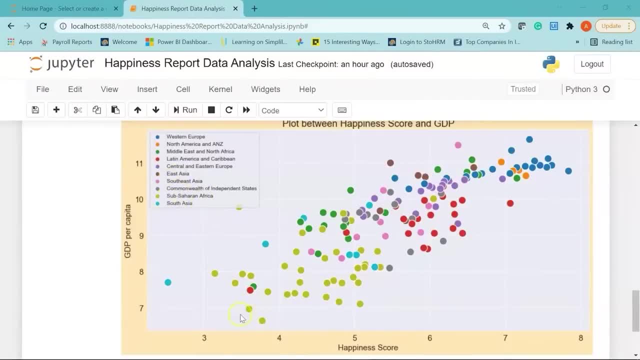 countries up here from the Sub Saharan Africa which have the lowest GDP per capita, but the happiness score is higher than this value or this country, so we can assume that this country is Afghanistan which has the lowest happiness score, as per the 2021 happiness report data. 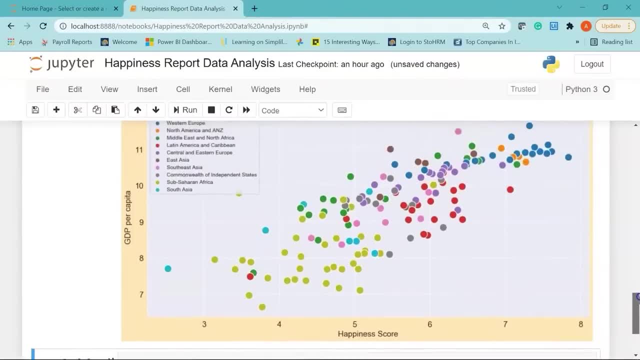 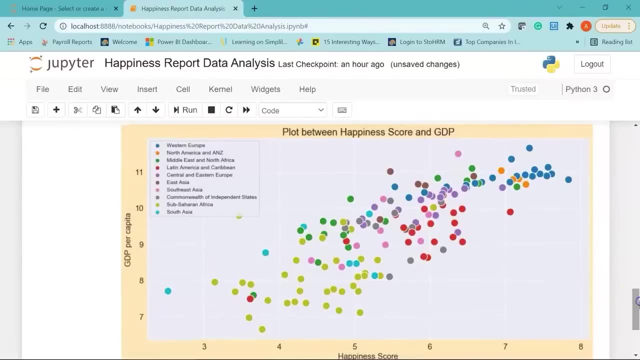 score from 0 to 8 and above, and on the y axis you have the gdp per capita and if you see, here in this region we have countries from western europe which have the highest happiness score and the gdp per capita is also the highest. 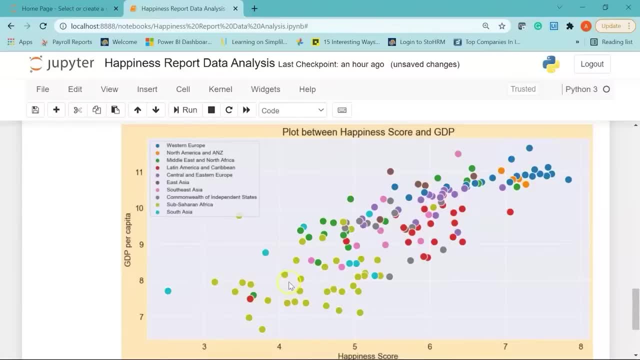 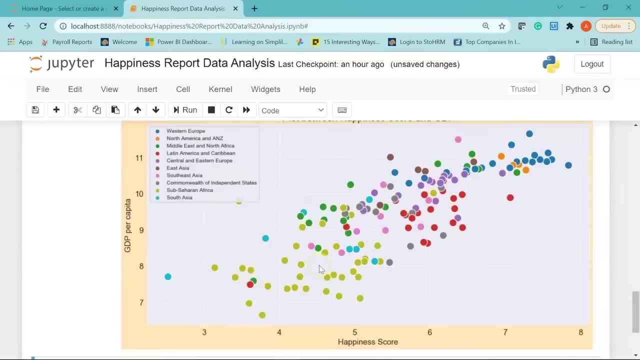 around this region. you can see here which is for green and in the legend you can see green is for sub saharan africa. so all these countries have low happiness score and even the gdp per capita is also low. and if you see the countries for latin america, 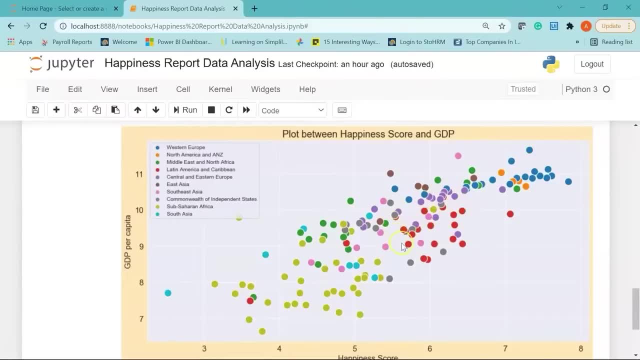 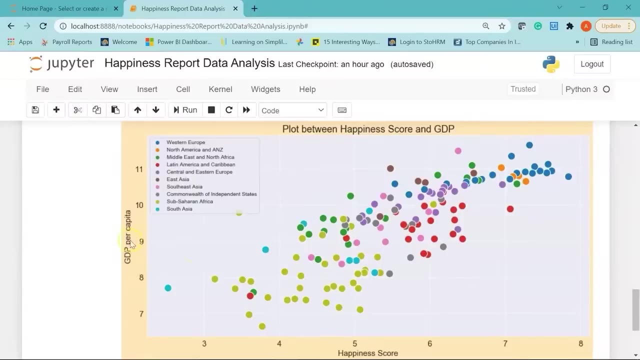 and caribbean. you see a lot of the values lie here. so they are all within the range of 5.5 to 7 in happiness score and even the gdp per capita is more than 9 for most of them. now even the happiness score is high for the countries that lie in the north america and ang region, and even that gdp per capita is also the highest. i can name a few countries such as australia, new zealand. we have canada and united states of america, which belong to the north america and ang region. cool, 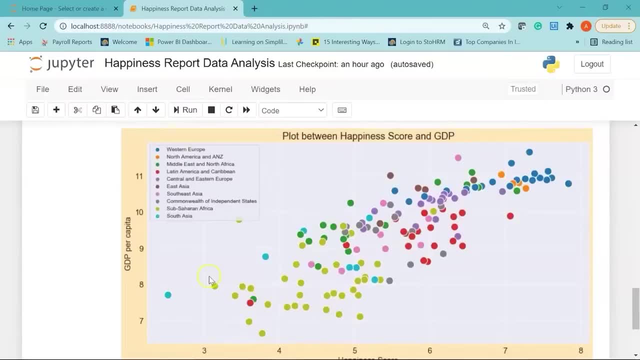 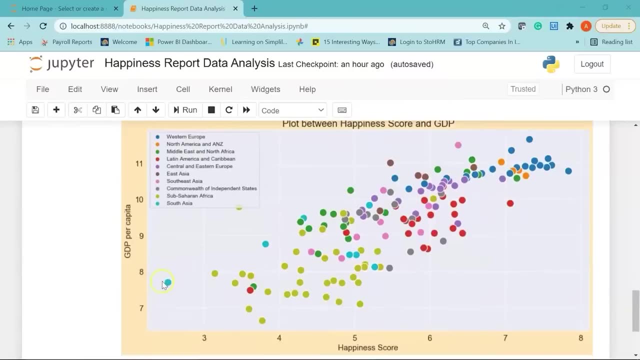 now there is one country which you see here. this seems to be like an outlier, which means that this is the country which has the lowest happiness score and even the gdp per capita is also low. but it is not the lowest because, you can see here, there are a few countries up here. 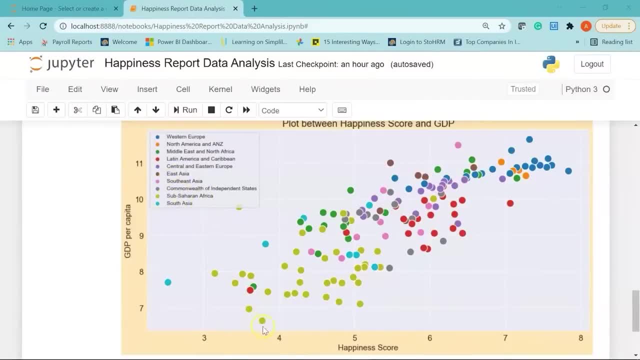 from the sub saharan africa which have the lowest gdp per capita, but the happiness score is higher than this value or this country, so we can assume that this country is afghanistan which has the lowest happiness score, as per the 2021 happiness report. 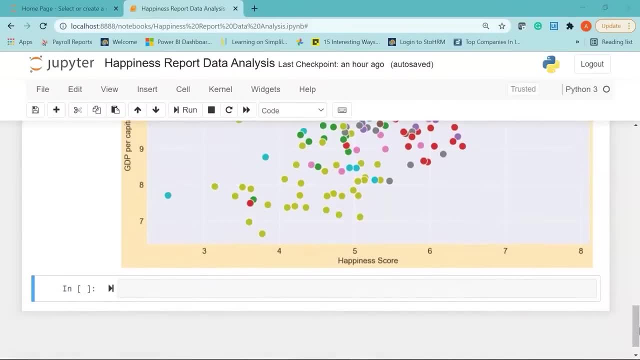 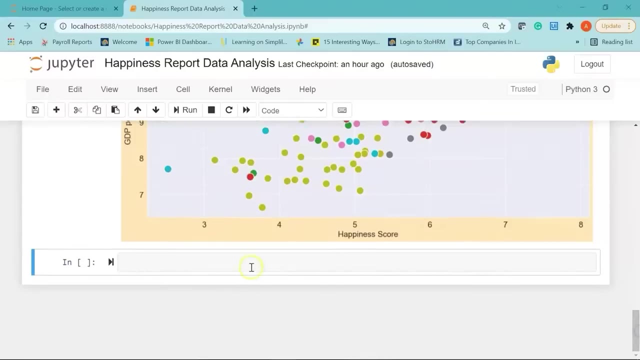 data. cool. now we will plot a pie plot to understand the gdp by region. so by this we can know which region has the highest percentage contribution to the world's gdp, as per our data. so for that i will create a variable gdp underscore region. 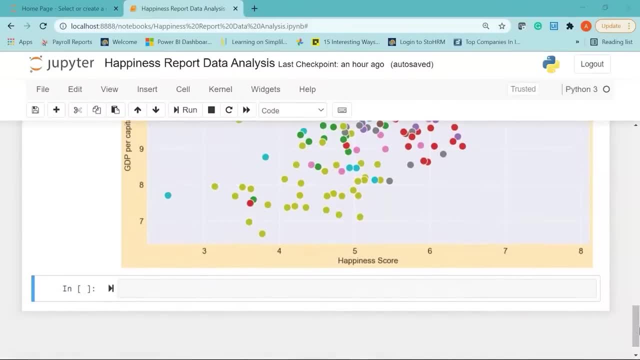 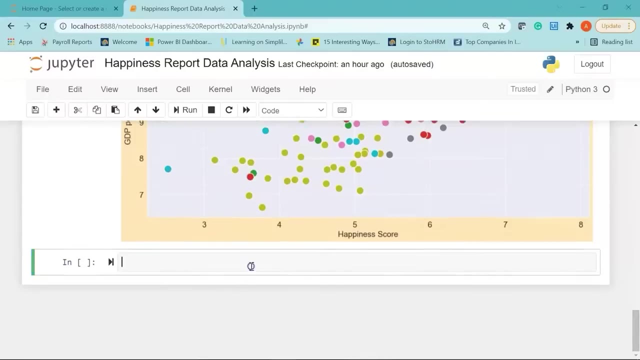 cool. now we will plot a plot to understand the GDP by region. so by this we can know which region has the highest percentage contribution to the world's GDP as per our data. for that I will create a variable GDP underscore region equal to. we will use our data frame. 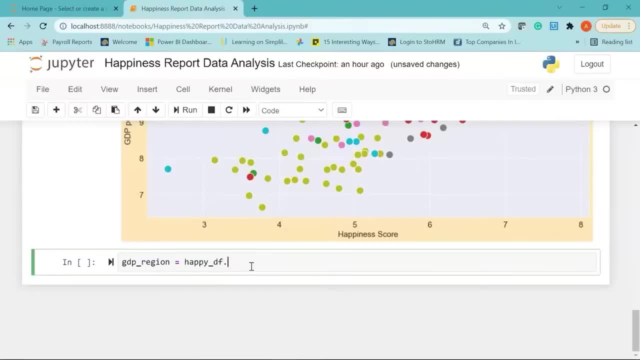 that is happy. underscore df dot. I am going to use the group by function and after that I am going to use my column. that is region. so we have named the column as regional underscore indicator. so I am going to group it by this region column and I am going to 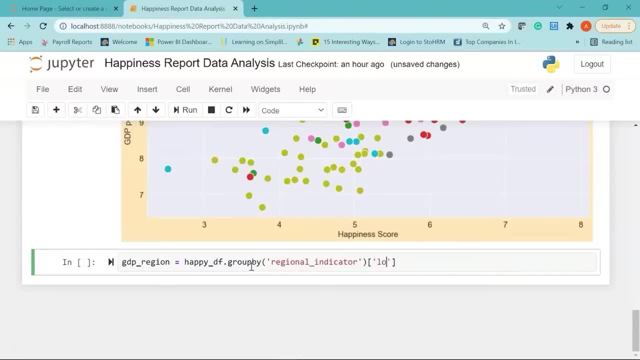 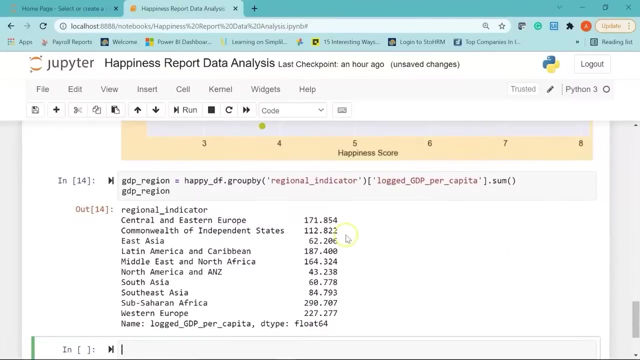 sum the values of GDP. so I am going to use the logged underscore GDP underscore per capita column and after that I am going to use the sum function and let me just print GDP underscore region. you can see it: here we have the sum of all the countries for different. 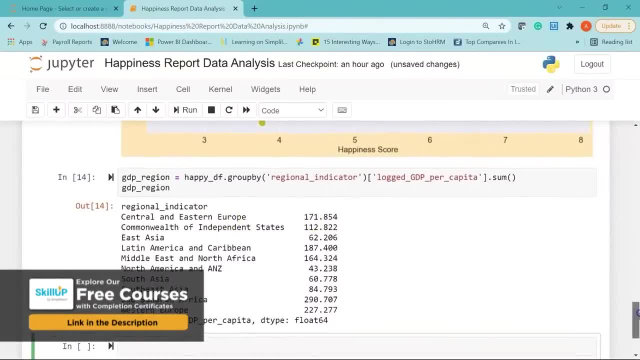 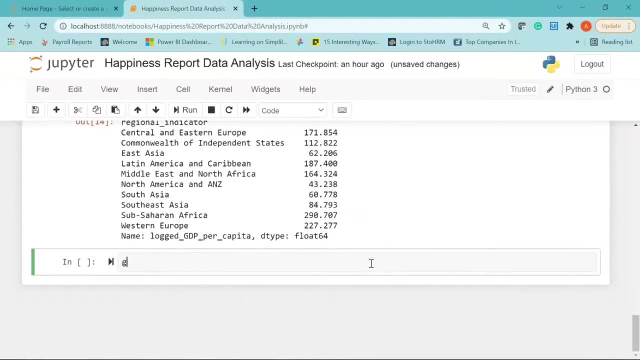 regions and their GDP all total. now this data, we are going to plot it in the form of a pi plot, so I will say GDP underscore, region, dot plot, dot pi. we are going to plot it in terms of percentage, so I am going to use a parameter called. 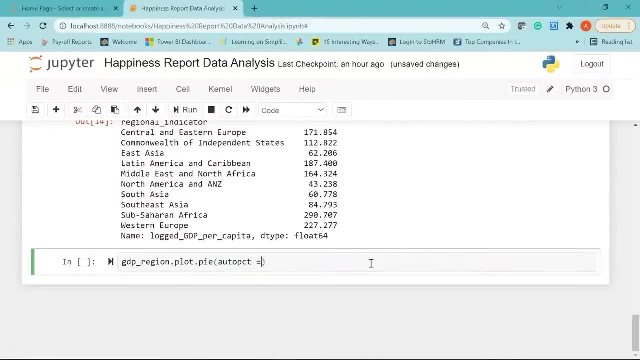 auto pct equal to. then I am going to pass in my format. so I will say percentage 1.1 of percentage percentage. then I will say plt dot. title. let's say the title of my pi plot is going to be GDP by region and I will say plt dot. 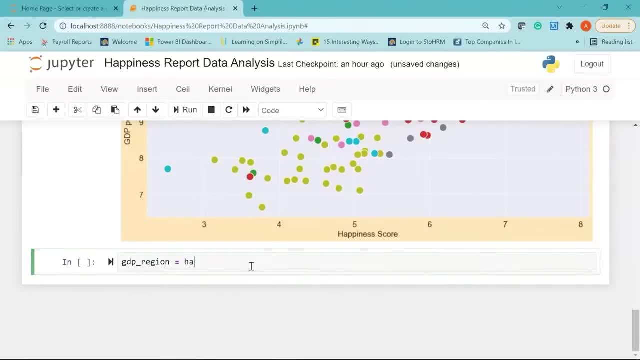 equal to. we will use our data frame. that is happy underscore df dot. i am going to use the group by function and after that i am going to use my column. that is region. so we have named the column as regional underscore indicator, so i am going to group it by this. 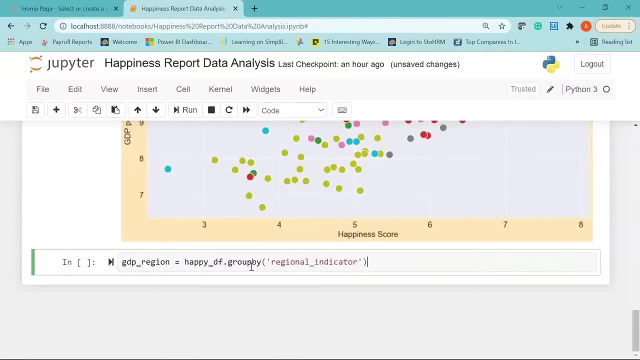 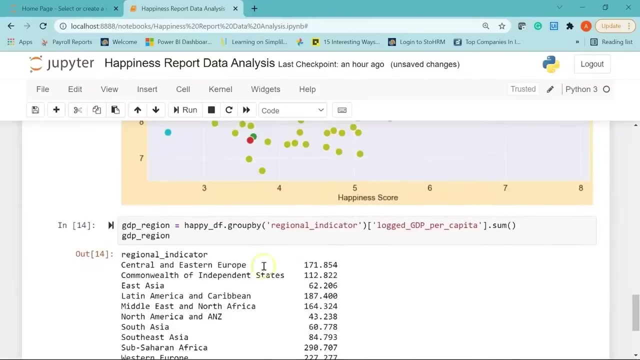 region column and i am going to sum the values of gdp. so i am going to use the logged underscore gdp underscore per capita column and after that i am going to use the sum function and let me just print gdp underscore region. you can see it here. 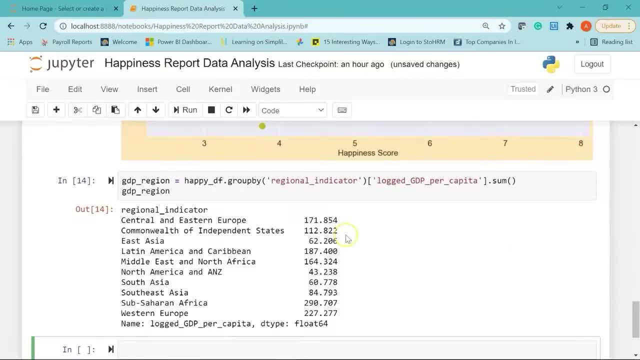 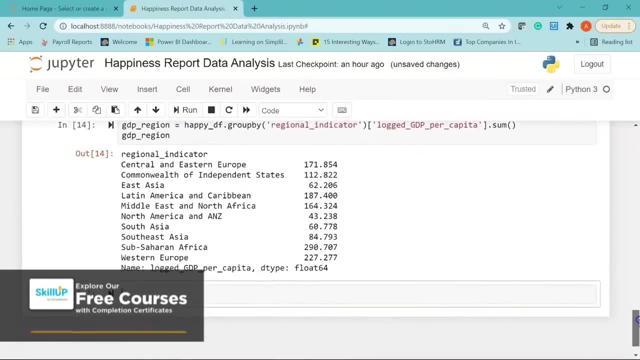 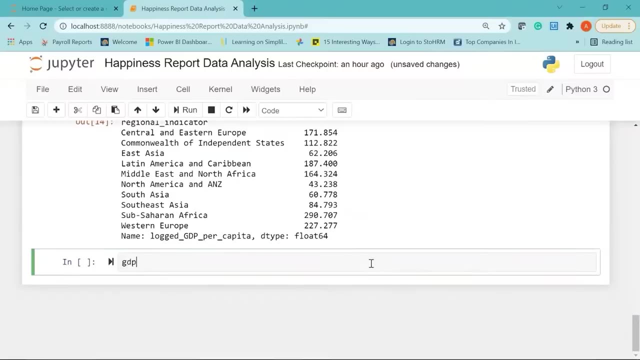 we have the sum of all the countries for different regions and their gdp all total. now this data, we are going to plot it in the form of a pie plot. so i will say gdp underscore region, dot plot, dot pie. we are going to plot it in terms of percentage. 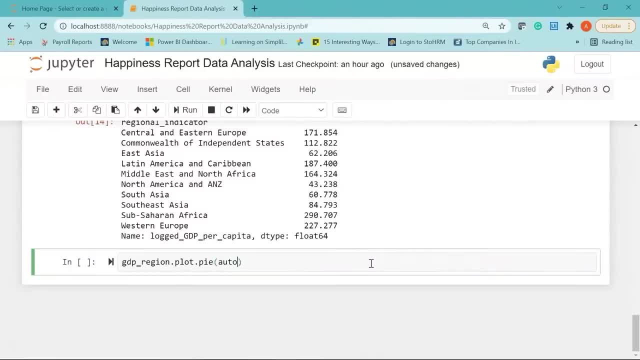 so i am going to use a parameter called auto pct equal to. then i am going to pass in my format. so i will say: percentage one dot, one f, percentage percentage. then i will say plt dot title. let's say the title of my pie plot is going to be: 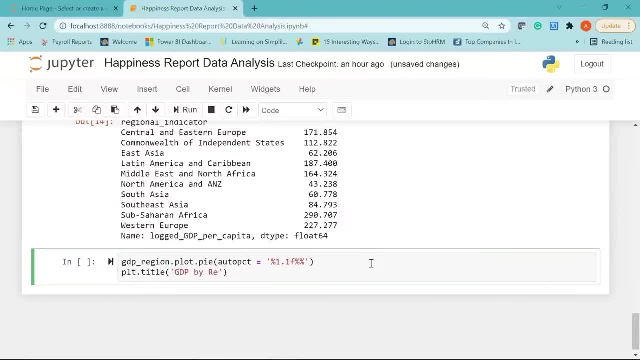 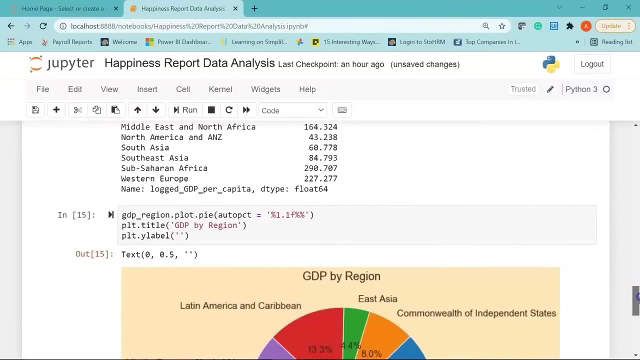 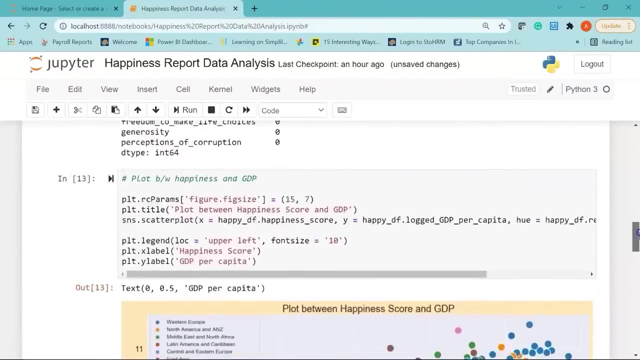 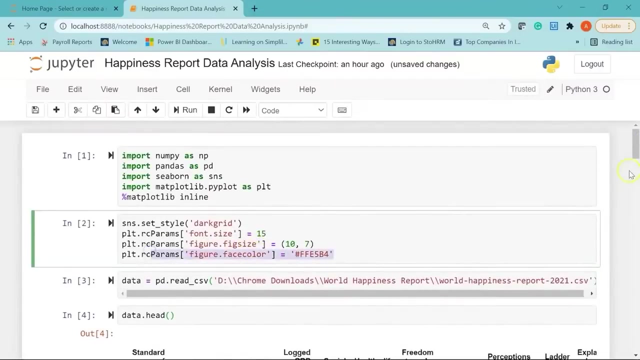 gdp by region and i will say plt, dot by label, which is going to be blank. let's run it ok. so here you can see we have the peach background at the back because we had assigned a peach face color. you can see it here. so for the first, 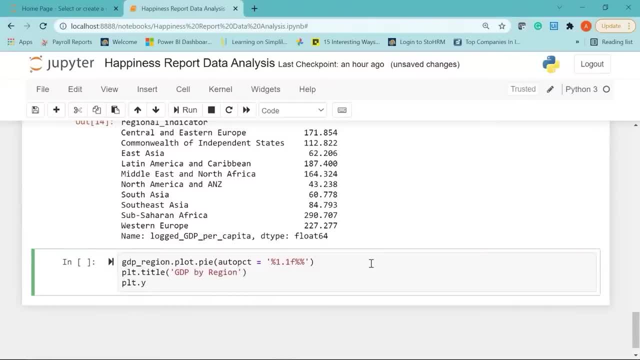 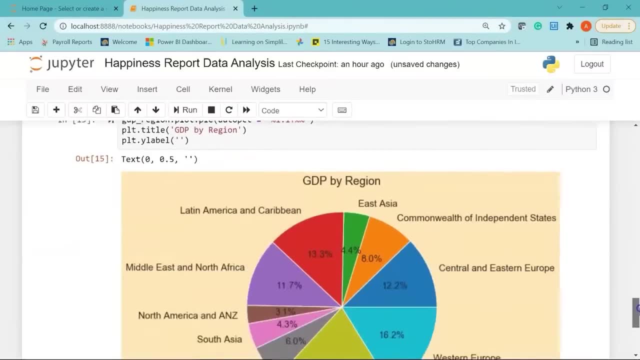 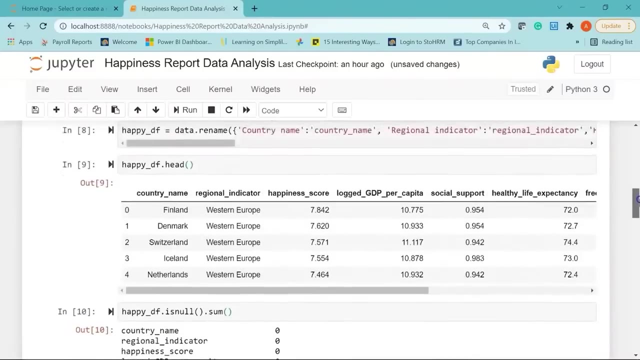 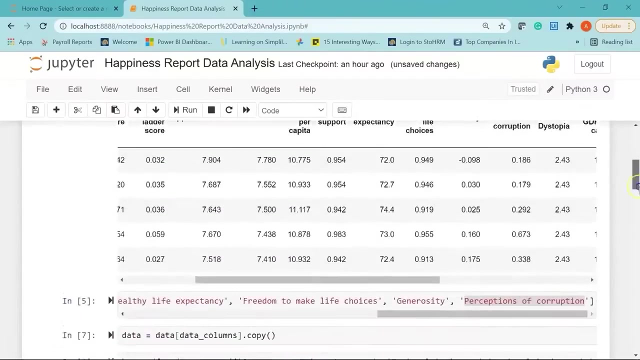 y label, which is going to be blank. let's run it ok. so here you can see we have the peach background at the back because we had assigned a peach face color. you can see it here. so for the first scatter plot also, we had the peach color at the 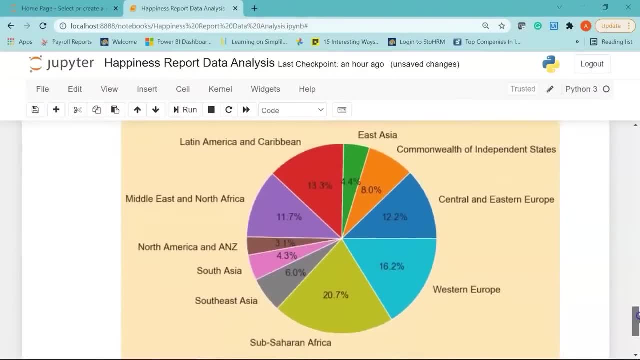 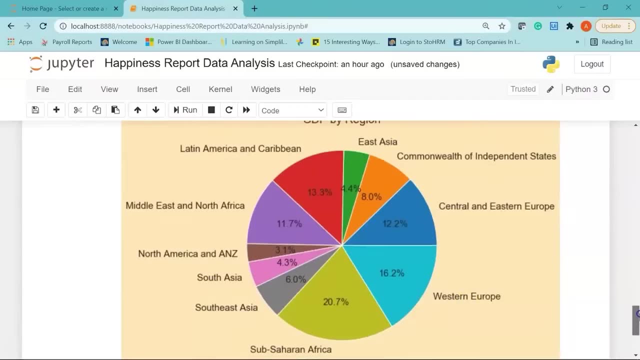 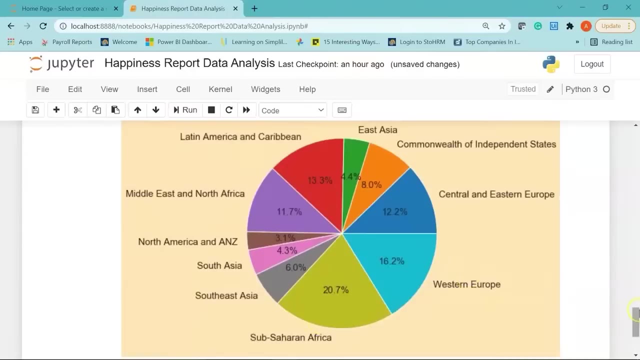 back and now you can see we have sub saharan Africa contributing 20.7% to the walls GDP, the reason being we have around 34 countries in the sub saharan Africa and we have the western European countries contributing to 16.2% of the GDP. 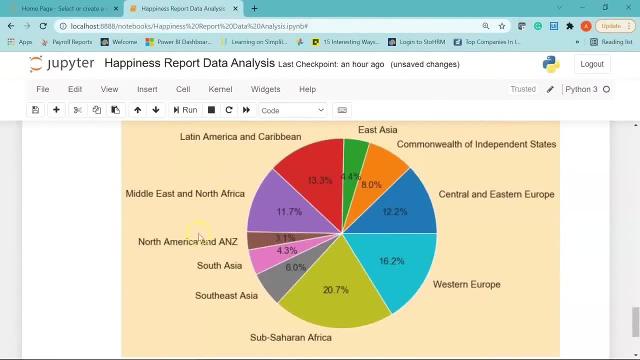 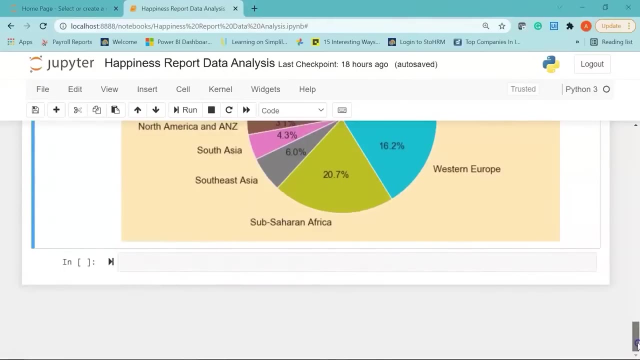 to check the list, we have North America and ANZ region because we only have 4 countries: America, Australia, Canada and New Zealand- so hence they are contributing only 3.1% to the walls GDP. ok, moving ahead, let's find the total number of countries in each. 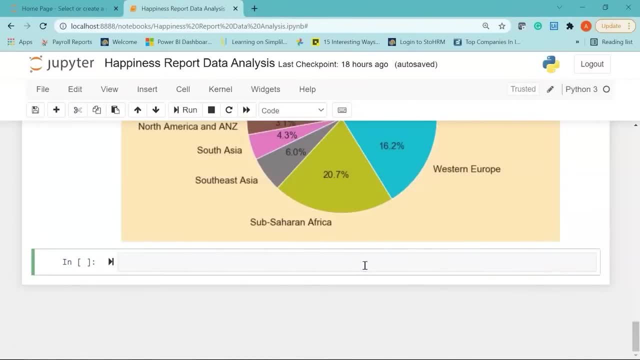 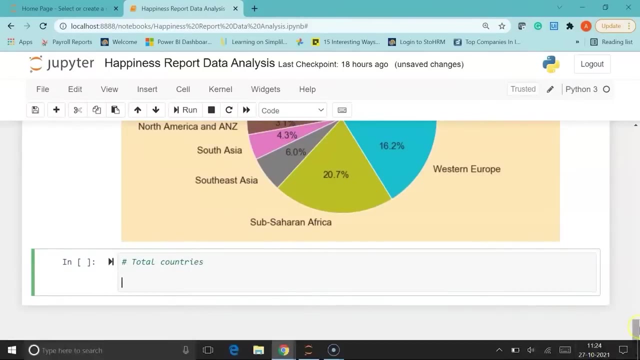 region. so for this we are going to use the group by function that is part of the pandas library, and we will count the total number of countries in each region. so I will just give a comment as total countries. alright, just scroll down. so I will create a variable called. 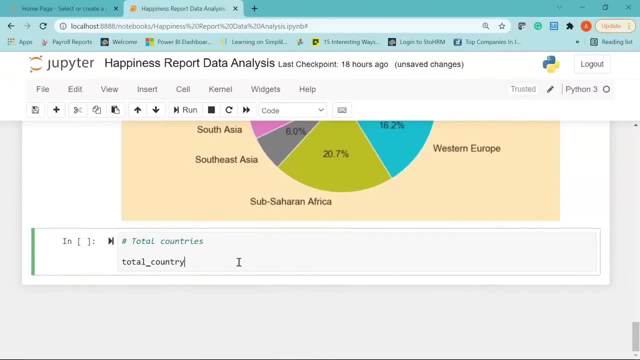 total underscore country. I am going to use my data frame that is happy underscore df dot. I am going to use the group by function. I will group the values based on the region column. so within single quotes I will say regional underscore indicator and then I am going to 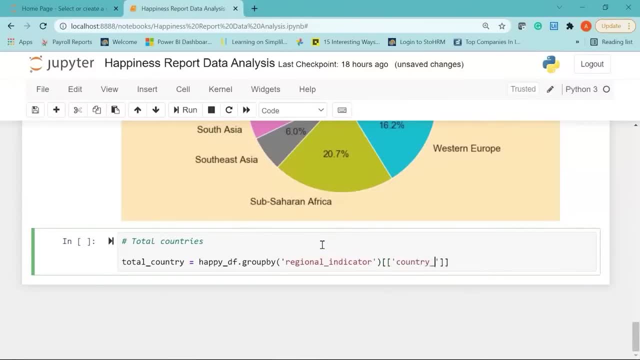 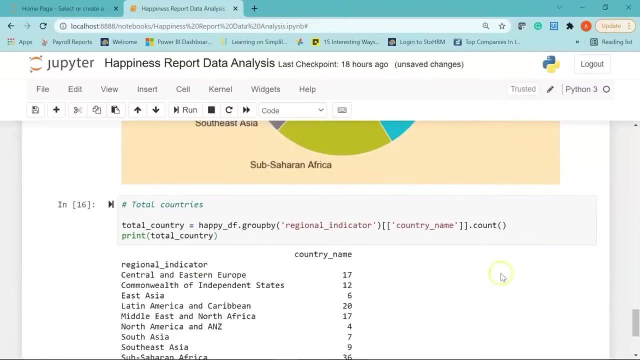 find the total count of country names. so I am using the column country underscore name and after that I will just use dot count. now let's go ahead and print my variable, that is total underscore country. alright, now let me hit shift, enter. ok, so here you can see. alright, so 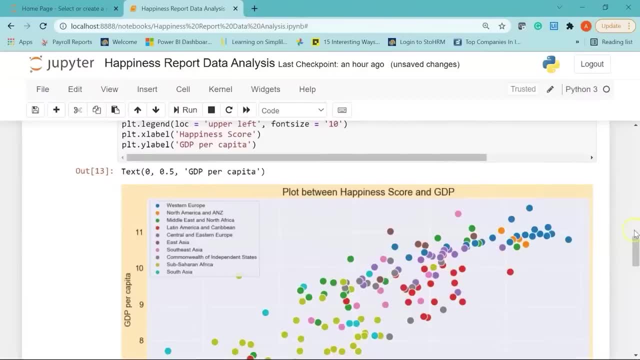 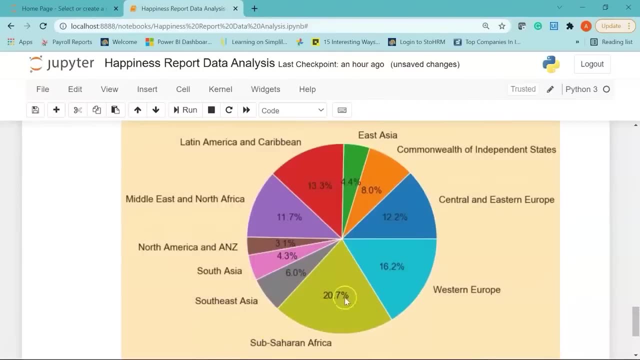 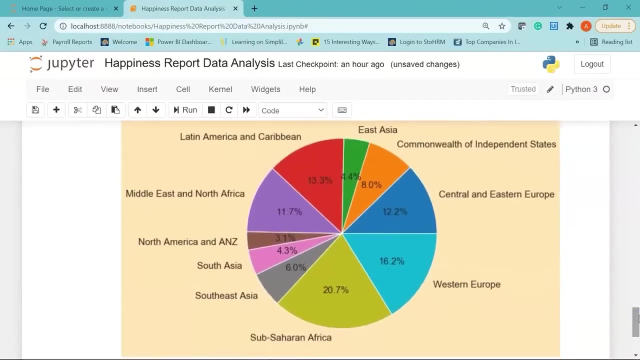 scatter plot. also, we had the peach color at the back and now you can see we have sub saharan africa contributing 20.7% to the world's gdp, the reason being we have around 34 countries in the sub saharan africa. 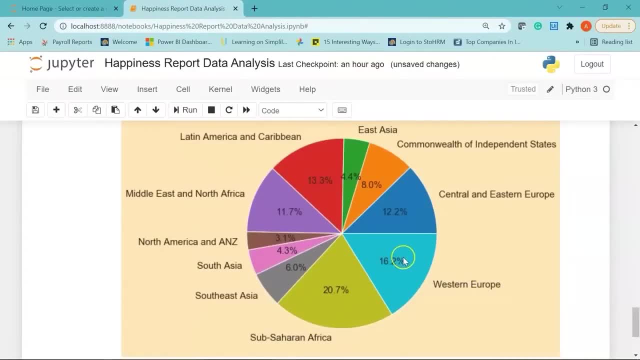 and we have the western european countries contributing to 16.2% of the gdp. to check the least, we have north america and anz region, because we only have 4 countries: america, australia, canada and new zealand- so hence they are contributing only 3.1% to the world's. 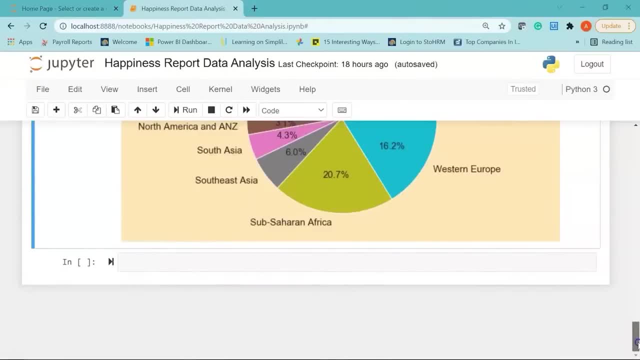 gdp. ok, now moving ahead, let's find the total number of countries in each region. so for this we are going to use the group by function that is part of the pandas library, and we will count the total number of countries in each region. so i will just give a comment. 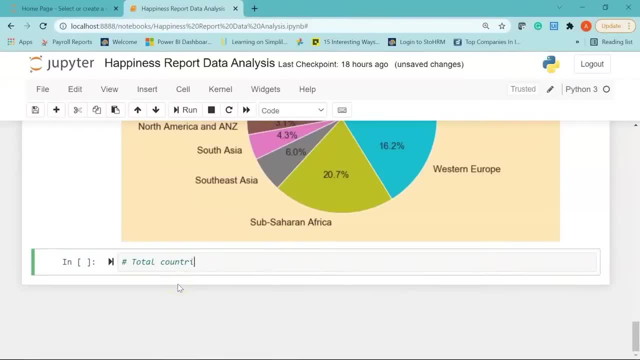 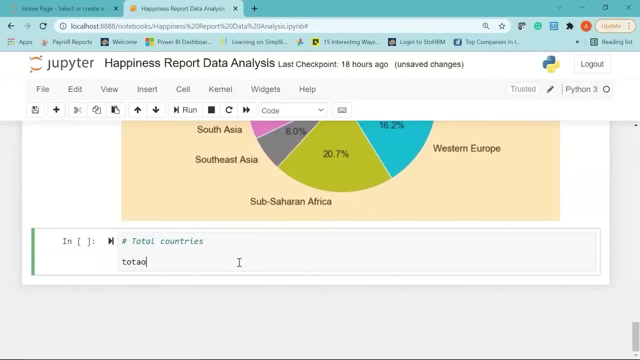 as total countries. alright, just scroll down. so i will create a variable called total underscore country. i am going to use my data frame that is happy, underscore df dot. i am going to use the group by function. i will group the values based on the region column, so within single. 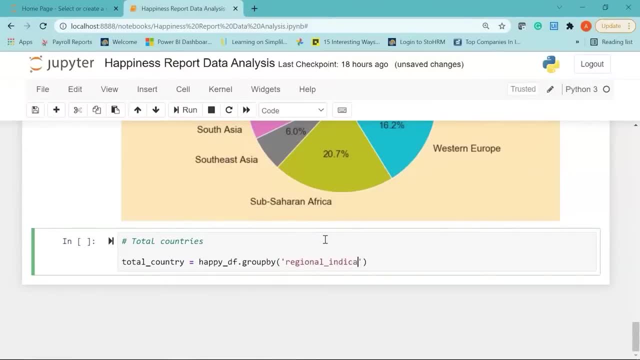 quotes, i will say regional underscore indicator and then i am going to find the total count of country names. so i am using the column country underscore name and after that i will just use dot count. now let's go ahead and print my variable, that is, total underscore country. 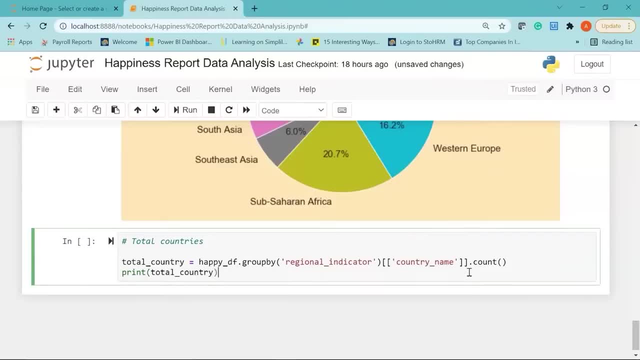 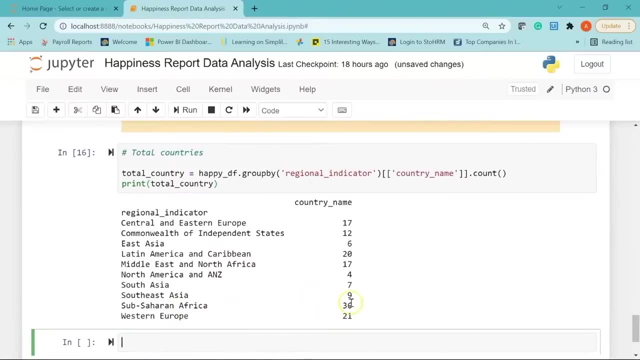 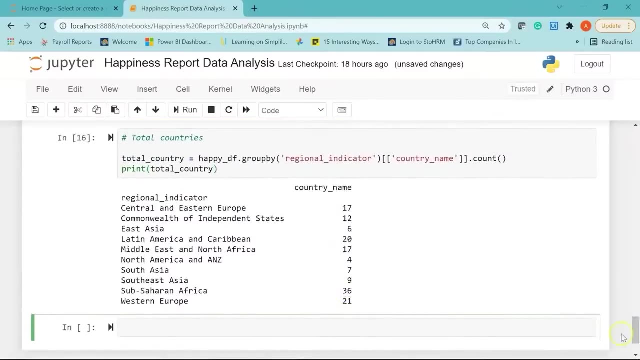 alright, now let me hit shift, enter. ok, so here you can see. alright, so for sub saharan africa there are total 36 countries and not 34, as i mentioned earlier. so hence you can see, because it has the highest number of countries, it is contributing the most. 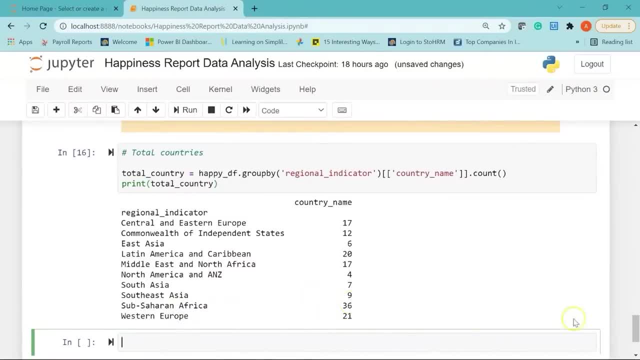 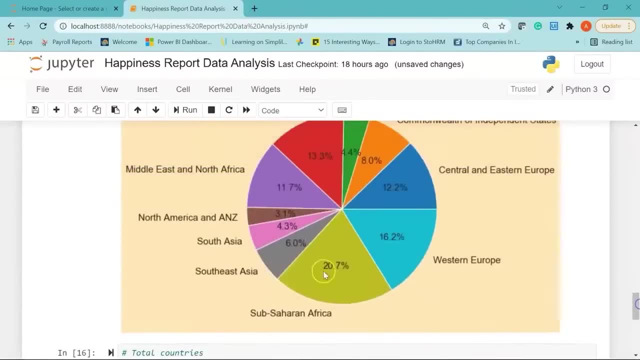 for sub saharan Africa, there are total 36 countries and not 34, as I mentioned earlier. so hence you can see, because it has the highest number of countries, it is contributing the most to the world's GDP, that is 20.7%. then we have: 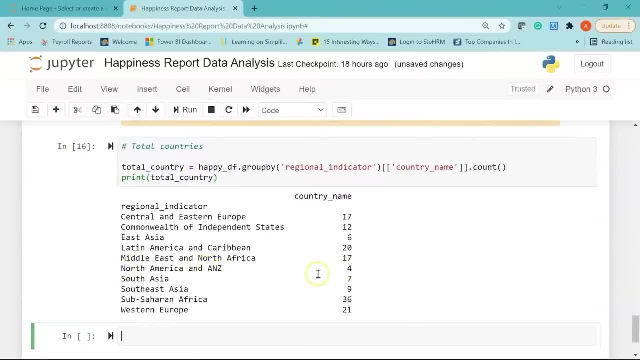 the least number of countries in North America and ANZ. that is only 4. we have 6 countries in East Asia and then we have 20 countries in Latin America and Caribbean, 12 countries in Commonwealth of Independent States, then we have 17 countries in Central. 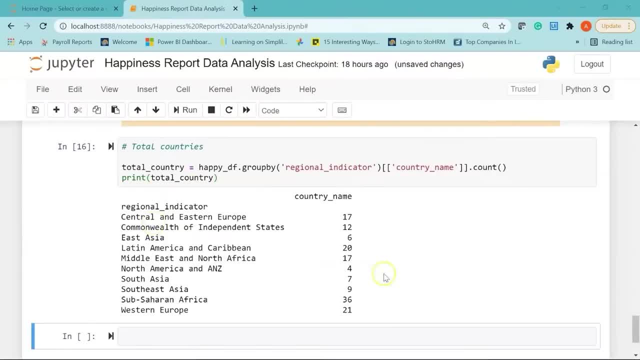 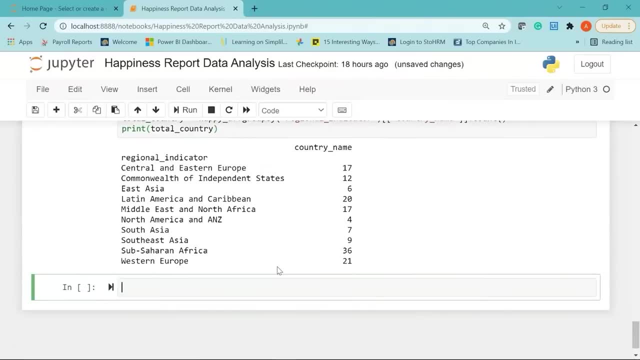 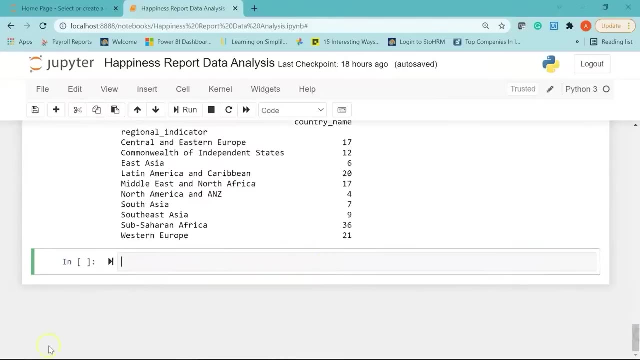 and Eastern Europe. cool, now I am going to show you how to create a correlation map so that we can see the relationship that exists between each of the variables that are present in our data set. I will just run through the code and we will see the output. 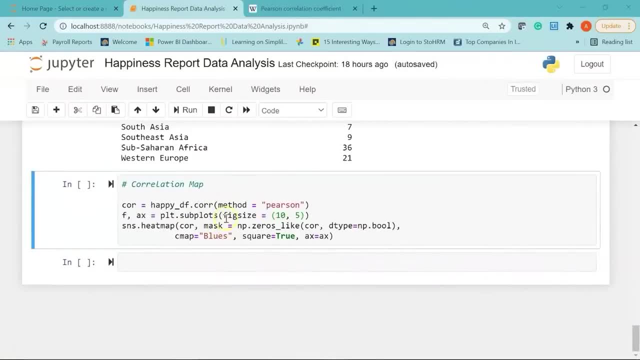 ok, so here I have my code written for the correlation map that I want to create. so first of all, I am going to compute the correlation matrix, so I have used the CORR function, which stands for correlation, and the method I am going to use is Pearson. 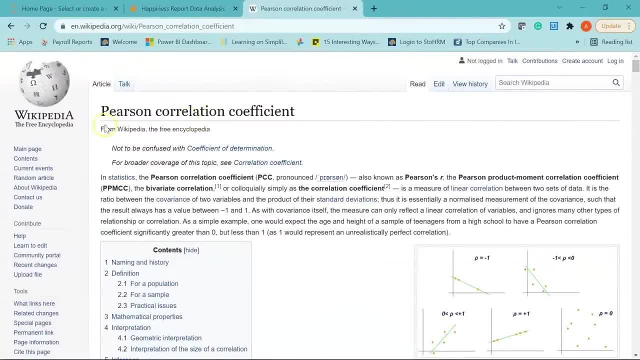 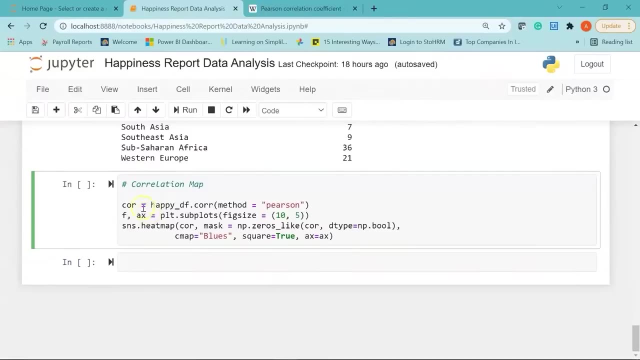 method. now here I have a Wikipedia page opened for Pearson correlation coefficient, so this is a nice article where you can understand what the Pearson correlation is all about. and then I am going to set up the matplotlib figures. so I have used the subplots function and I have given the figure. 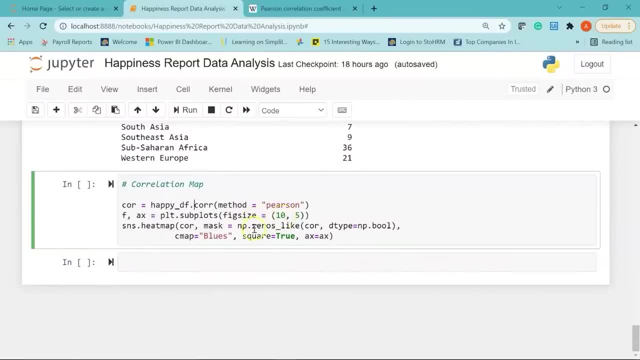 size as 10,5, and after that we are going to draw the heat map with the mask. so I am using the heat map function present in the Seaborn library and then I have passed in my variable, that is COR, which essentially stands for correlation. 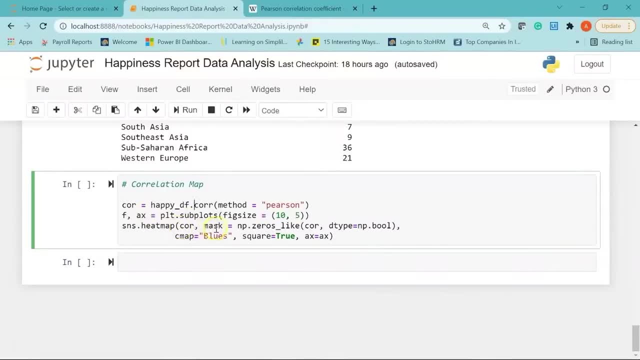 and then I have used mask, which is a Boolean array or it can be a data frame and it is an optional parameter. if it is passed, the data will not be shown in cells where the mask is true and the cells with missing values are automatically masked. after that, I have 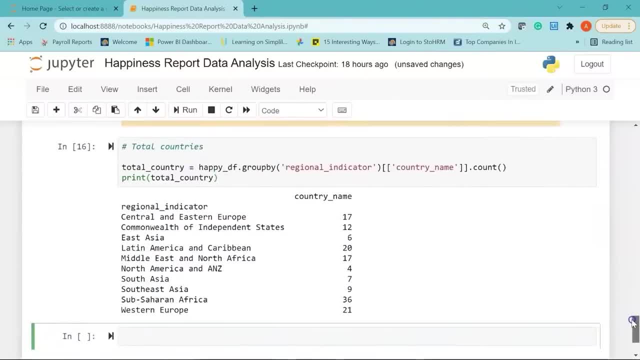 to the world's gdp, that is 20.7%. then we have the least number of countries in north america and ang, that is only 4. we have 6 countries in east asia and then we have 20 countries in latin america and caribbean, 12 countries in 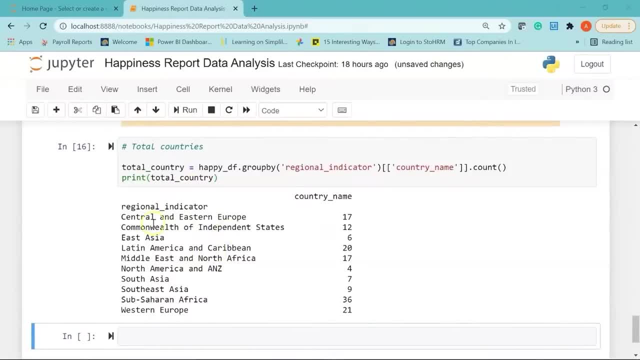 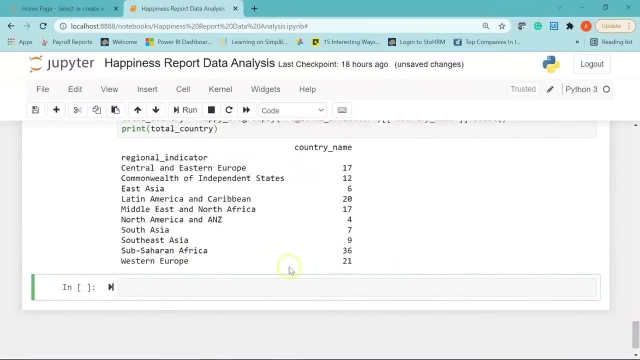 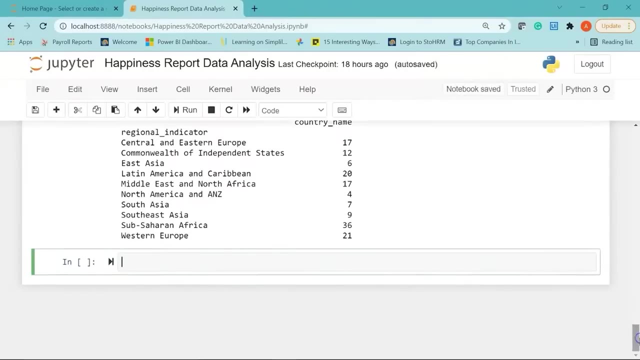 commonwealth of independent states. then we have 17 countries in central and eastern europe. cool, now i am going to show you how to create a correlation map so that we can see the relationship that exists between each of the variables that are present in our data set. i will just run through the 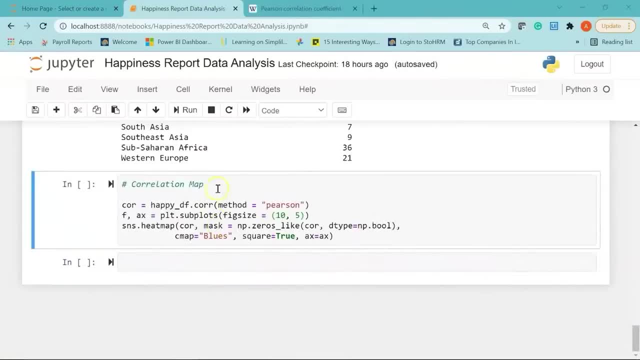 code and we will see the output. ok, so here i have my code written for the correlation map that i want to create. so first of all, i am going to compute the correlation matrix. so i have used the corr function, which stands for correlation, and the method i am going to use is: 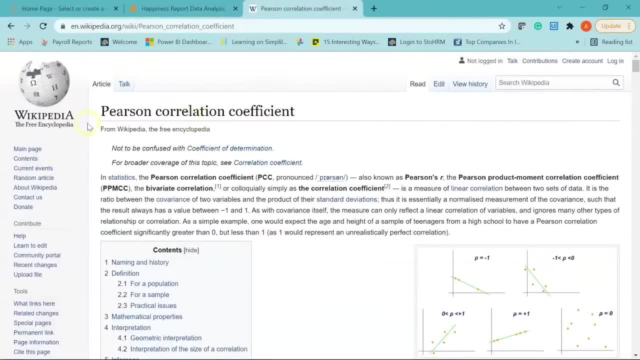 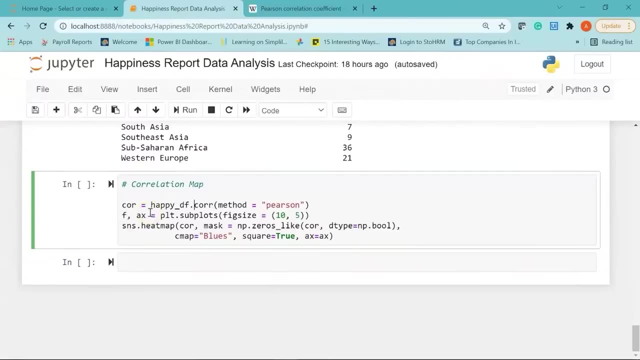 pearson method. now here i have a wikipedia page opened for pearson correlation coefficient, so this is a nice article where you can understand what the pearson correlation is all about. and then i am going to set up the matplotlib figures. so i have used the subplots function and i have given the 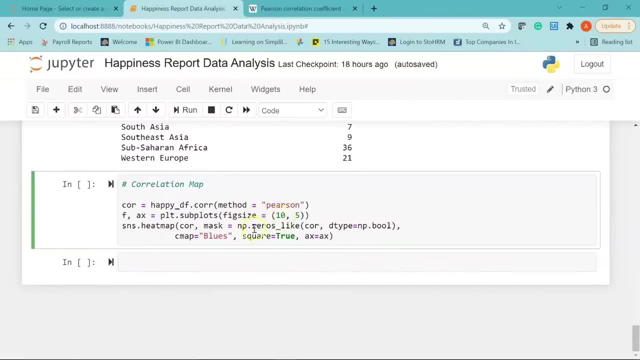 figure size as 10,5, and after that we are going to draw the heat map with the mask. so i am using the heat map function present in the seaborn library, and then i have passed in my variable, that is cor, which essentially stands for correlation, and then 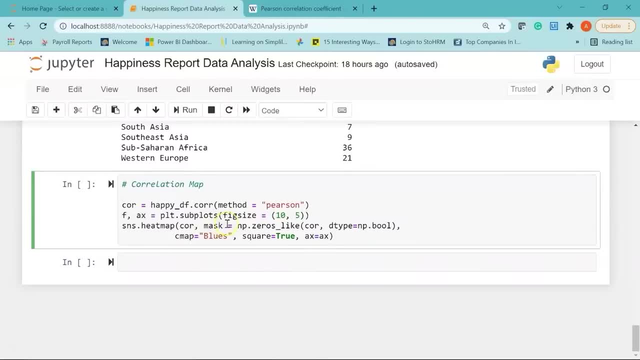 i have used mask, which is a boolean array or it can be a data frame and it is an optional parameter. if it is passed, the data will not be shown in cells where the mask is true and the cells with missing values are automatically masked. after that, i have used the. 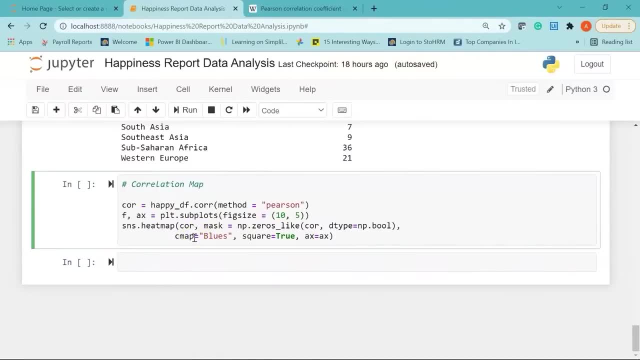 cmap parameter, which stands for color map, so you can customize the colors in your heat map. and i am going to create a heat map which is in square shape, so i have set square equal to true and the axis i am going to pass it as ax, which i have. 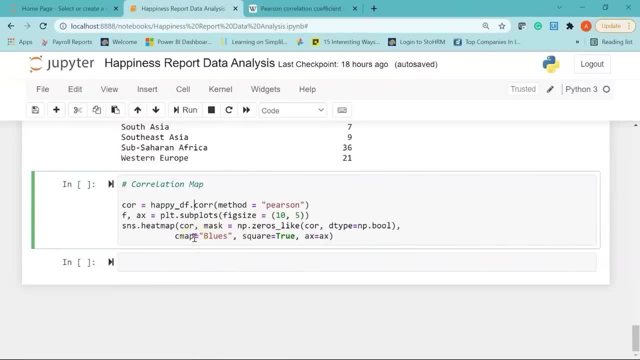 used the CMAP parameter, which stands for color map, so you can customize the colors in your heat map, and I am going to create a heat map which is in square shape, so I have said square, equal to true, and the axis I am going to pass it as AX, which I have. 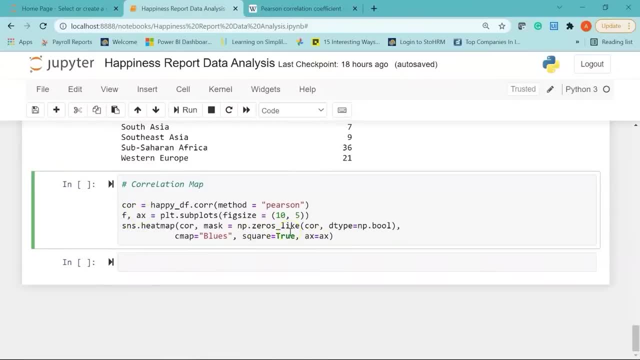 defined here. so this is the matplotlib axis and it is optional, so axis in which you want to draw the plot. otherwise you can use the current relative axis. now let me just go ahead and run this and we will see the heat map. there you go. so if I scroll down, 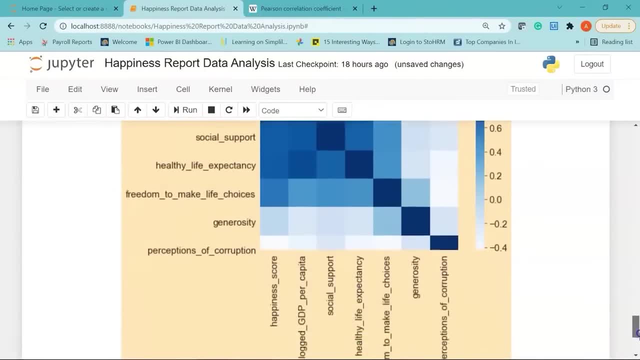 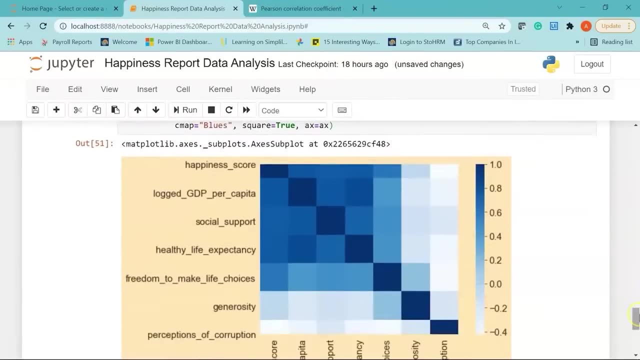 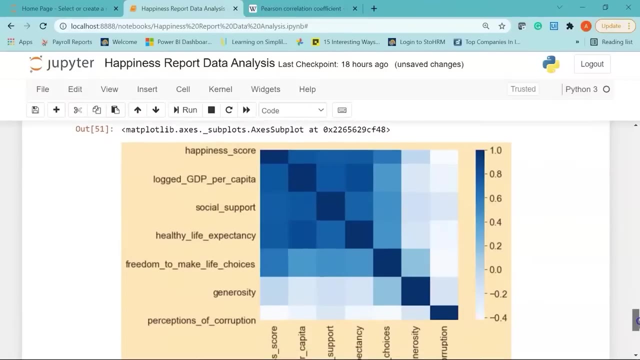 here we have the correlation matrix and since I had given my CMAP as blue and here you can see it is mostly blue and we have the scale here, now I will tell you how to read this correlation matrix. so wherever the cells are in blue or dark blue color, this 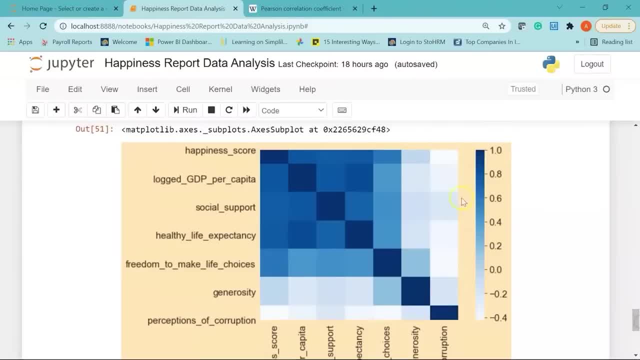 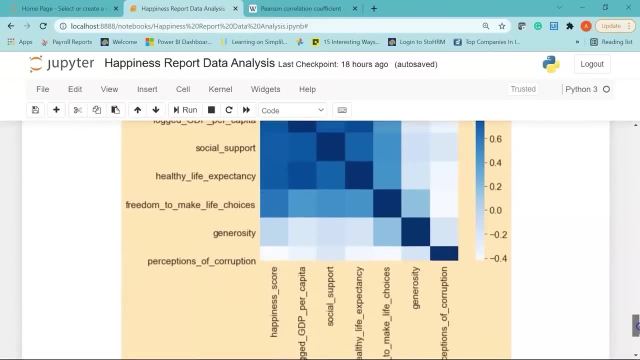 means that the variables have very high correlation. and all this cells where you see light blue color or grayish and white color. this indicates that the variables have very low correlation. for example, there is very low or almost negative correlation between happiness score and perceptions of corruption. so obviously, if the citizens of a country 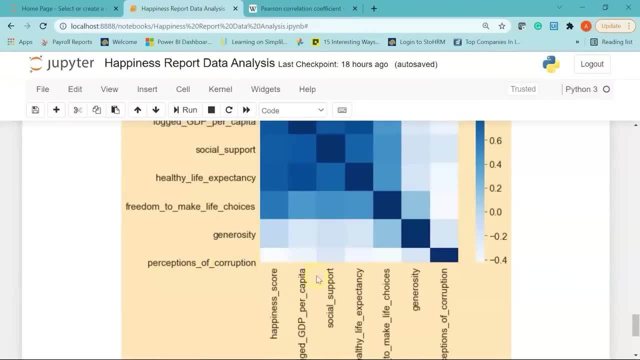 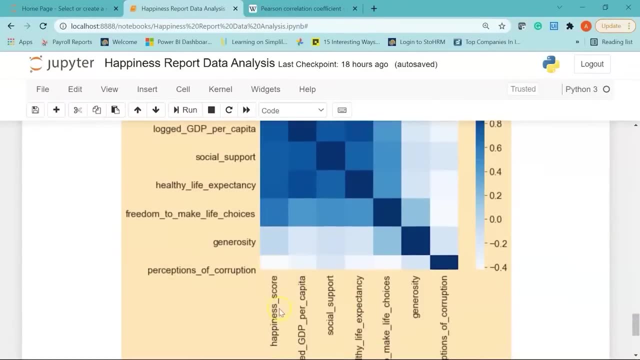 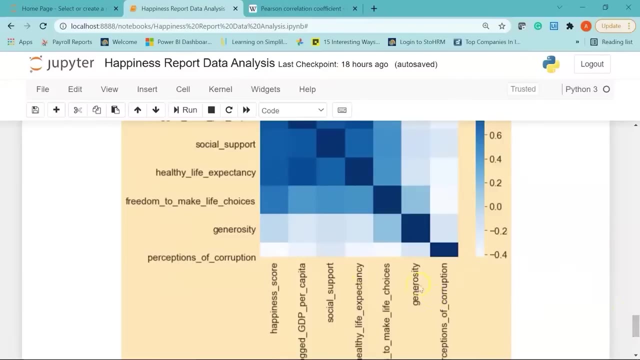 feel that there is a lot of corruption in the country, their happiness score would obviously be less or low. and if you see, there is also low correlation between happiness score and generosity. there is again low correlation between health, life expectancy and perceptions of corruption. and if you see, these places, 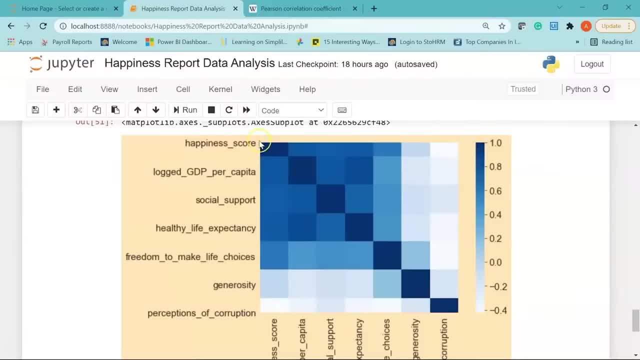 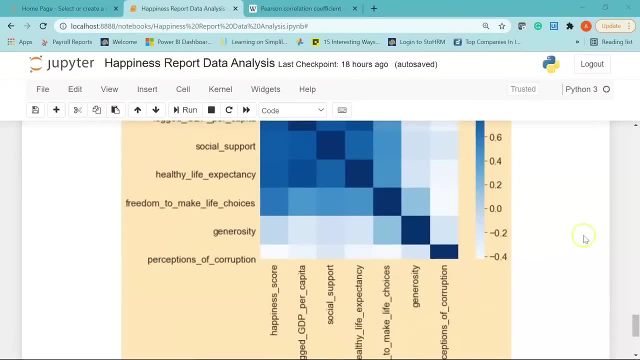 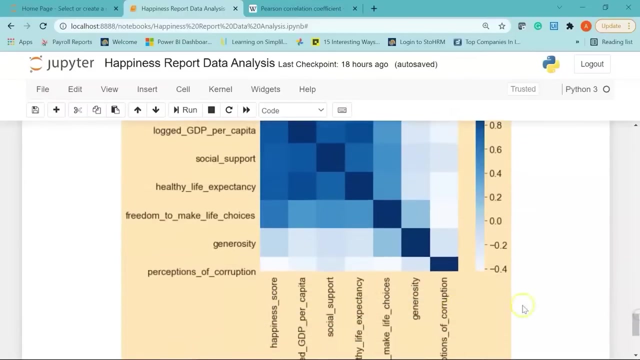 there is really high correlation between the happiness score and GDP per capita. again, for social support also, there is very high correlation. now, if you see, even for social support and healthy life expectancy there is very high correlation, but there is low correlation between making life choices and generosity. 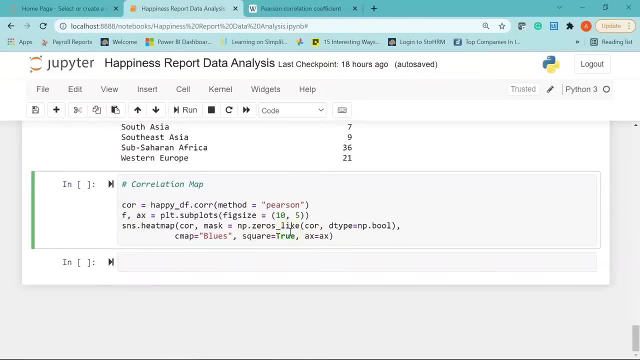 defined here. so this is the matplotlib axis and it is optional, so axis in which you want to draw the plot. otherwise you can use the current active axis. now let me just go ahead and run this and we will see the heat map. there you go. so if i scroll, 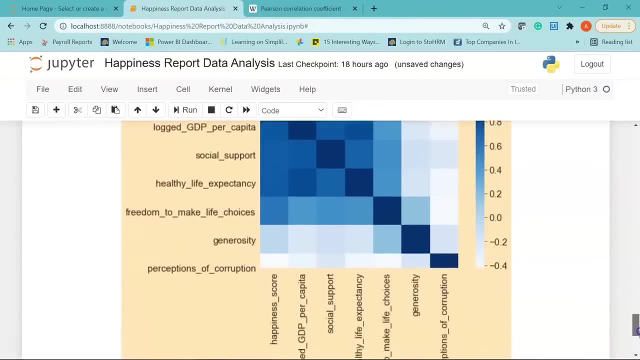 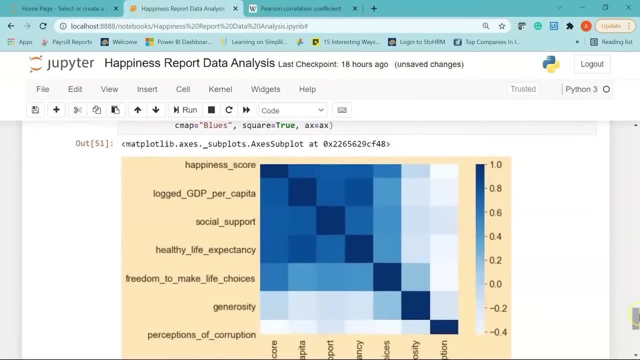 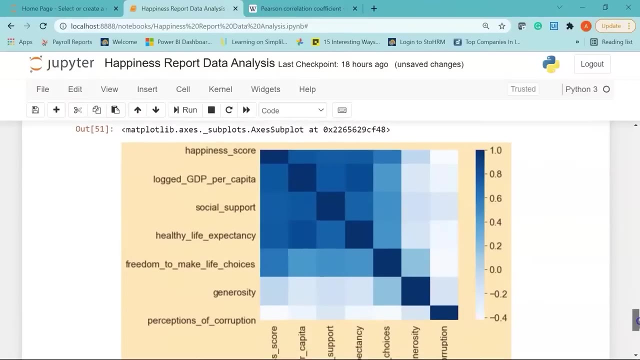 down here we have the correlation matrix and since i had given my c map as blue and here you can see it is mostly blue and we have the scale here, now i will tell you how to read this correlation matrix. so wherever the cells are in blue or dark blue color, 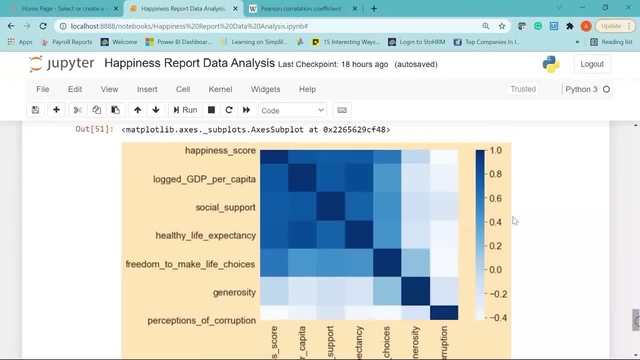 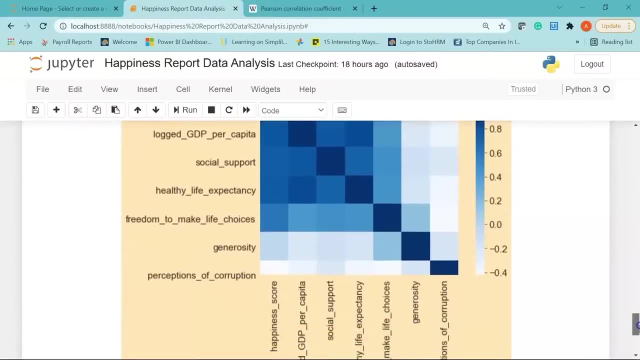 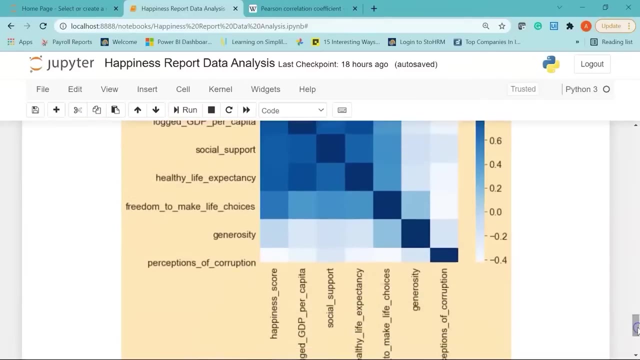 this means that the variables have very high correlation and all these cells where you see light blue color or grayish and white color. this indicates that the variables have very low correlation. for example, there is very low or almost negative correlation between happiness score and perceptions of corruption. 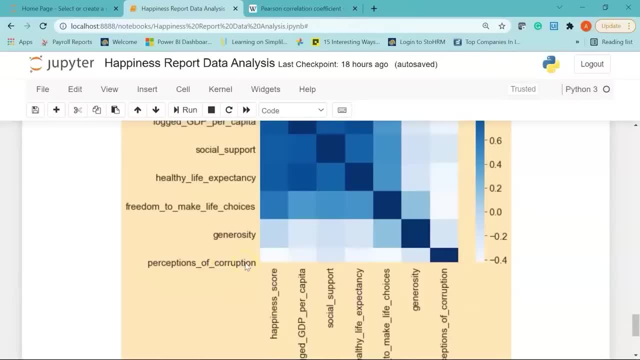 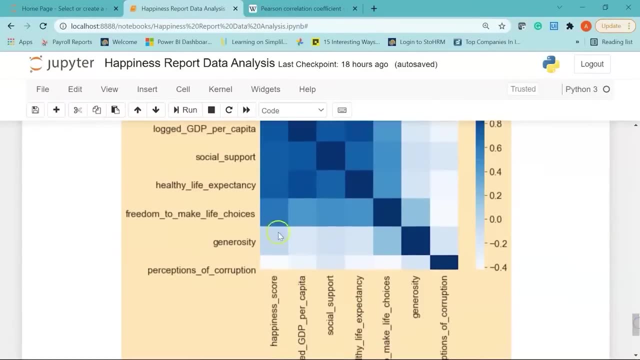 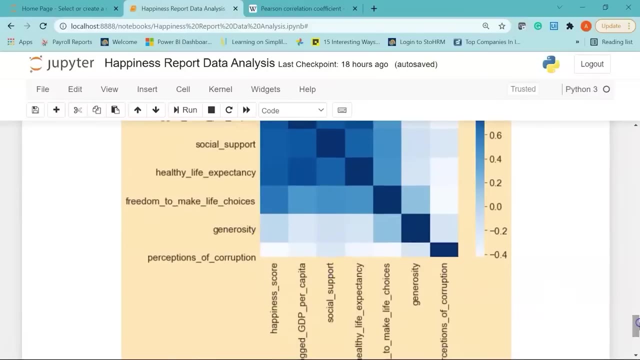 so obviously, if the citizens of a country feel that there is a lot of corruption in the country, their happiness score would obviously be less or low. and if you see, there is also low correlation between happiness score and generosity. there is again low correlation between health, life expectancy and 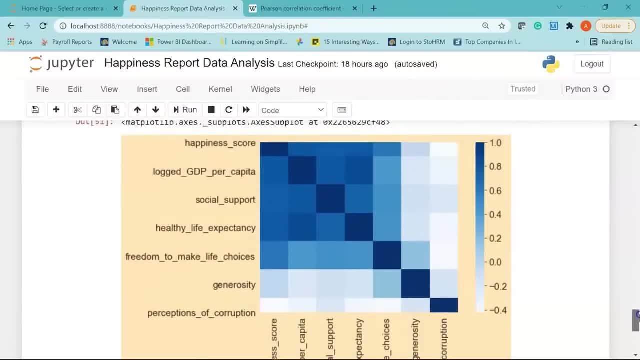 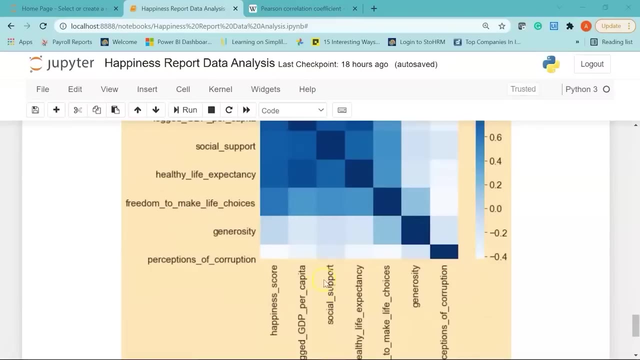 perceptions of corruption and if you see, these places there is really high correlation between the happiness score and GDP per capita. again, for social support also, there is very high correlation. now, if you see, even for social support and healthy life expectancy there is very high correlation, but there is. 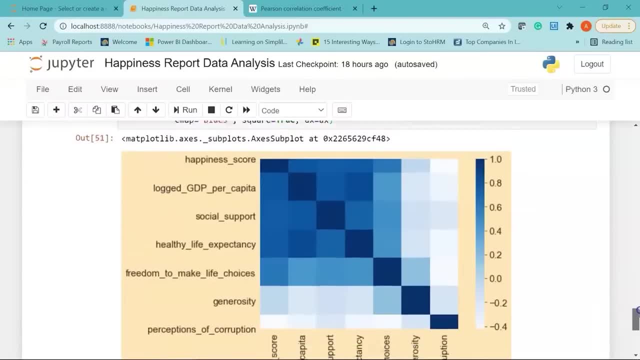 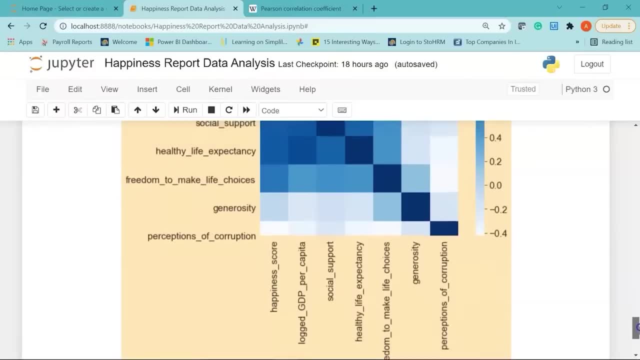 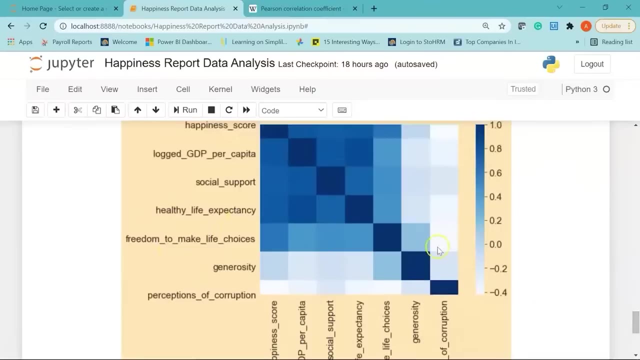 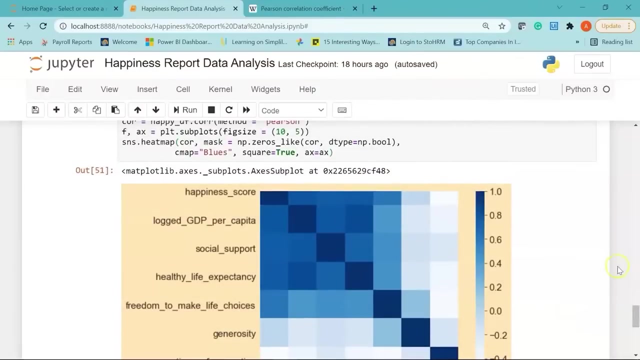 low correlation between making life choices and generosity and there is negative correlation between corruption and freedom of making life choices. you can see it is almost white color, which means it falls around this region, so negative correlation. similarly, for logged GDP per capita and corruption, there is negative correlation. 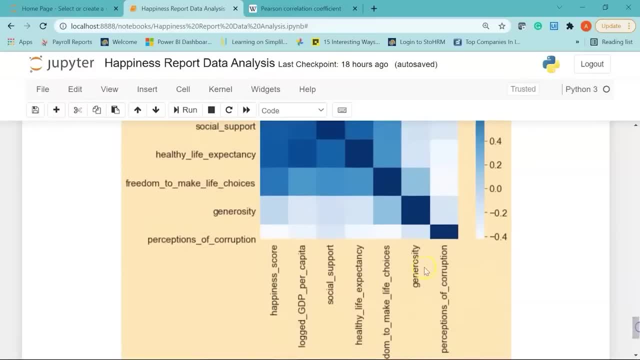 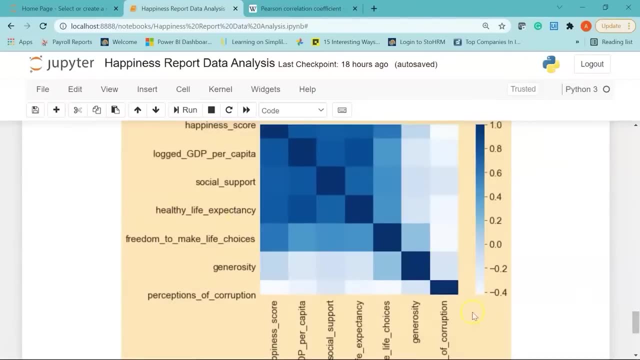 and there is negative correlation between corruption and freedom of making life choices. you can see it is almost white color, which means it falls around this region, so negative correlation. similarly, for logged GDP per capita and corruption, there is negative correlation. alright, ok, now we are going to visualize. 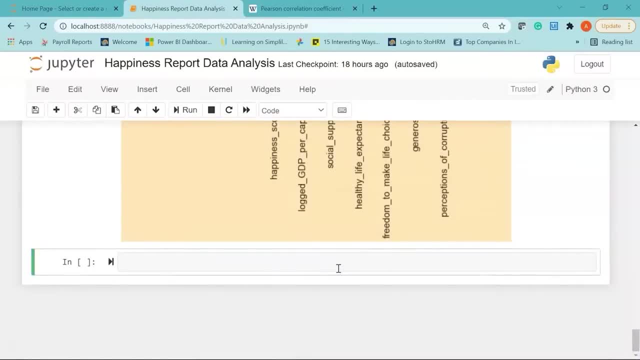 a bar plot that will tell us the corruption in different regions. so i will just give a comment: corruption in regions. let me just scroll down, ok, so i will create a variable called corruption, which will be equal to my data frame. that is happy underscore df. now, first of all, i am going to use 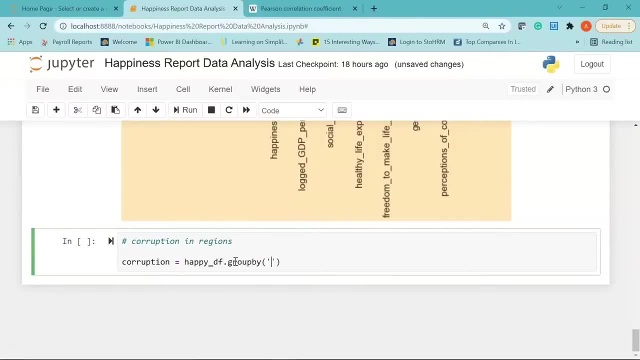 the group by function, to group all my regions. so i will say regional underscore indicator, which is my column name present in the dataset, and after this i am going to find the average of the corruption, that is, perceptions of corruption. so i am going to pass in my 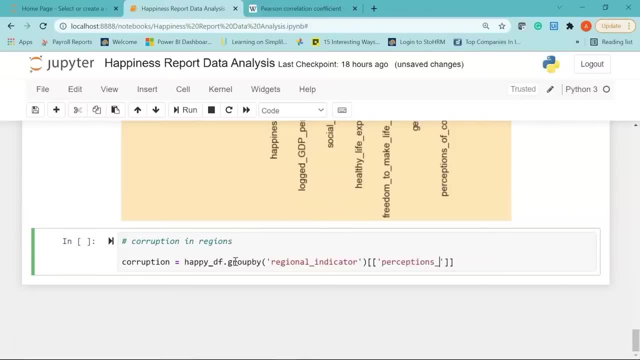 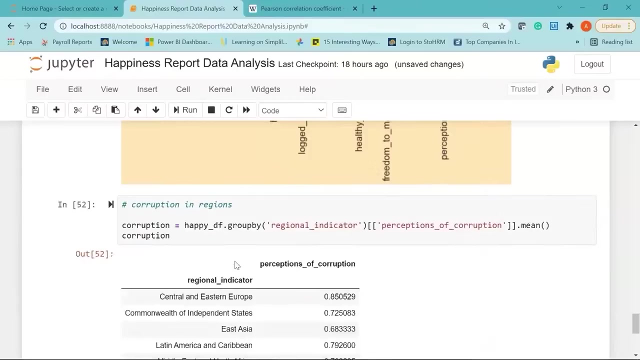 variable name, that is, perceptions of corruption, and i am going to use the mean function to find the average corruption in each of these regions. now let me just go ahead and print my variable that is corruption. if i run it, you can see. here i have the values for. 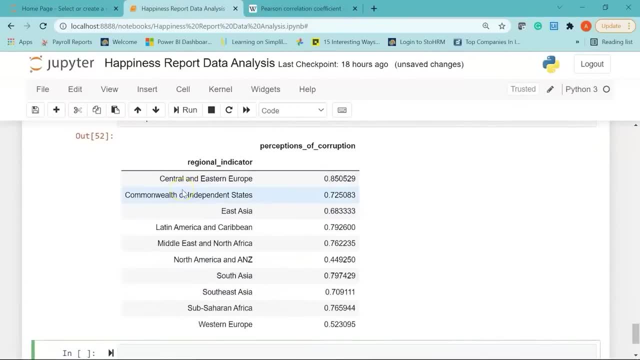 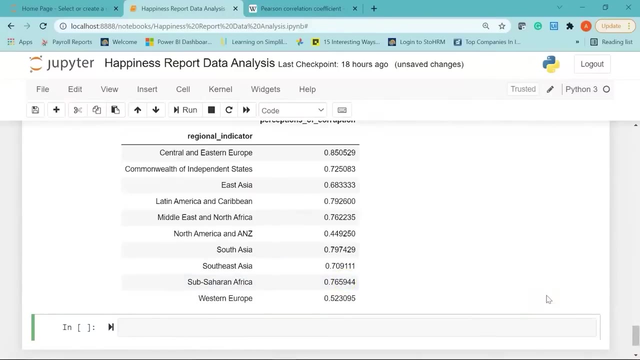 the different regions and from here you can see that central and eastern europe has the highest perceptions of corruption, as per the questions answered in the poll, and if you see the table, we have western europe and the north america region with the least perceptions of corruption. now we are going to visualize this. 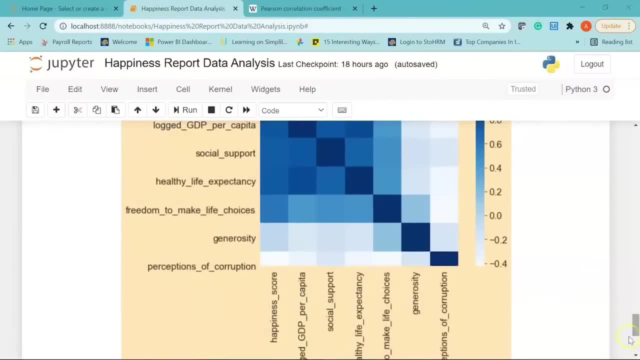 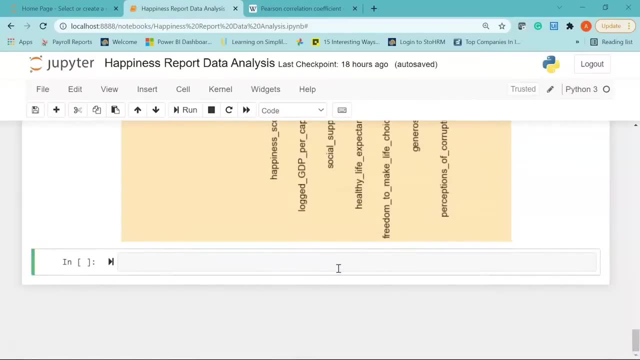 alright. ok, now we are going to visualize a bar plot that will tell us the corruption in different regions. so I will just give a comment: corruption in regions. let me just scroll down. ok, so I will create a variable called corruption, which will be equal to my. 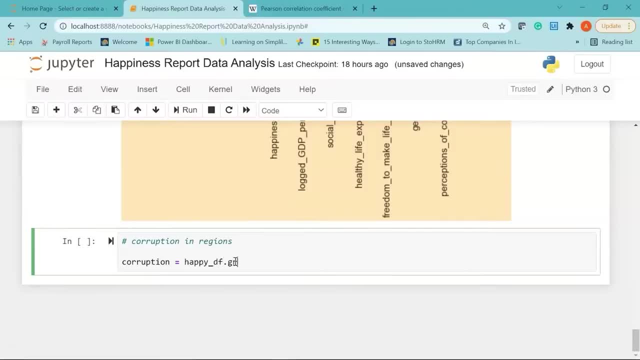 data frame. that is happy underscore df. now, first of all, I am going to use the group by function to group all my regions. so I will say regional underscore indicator, which is my column name present in the data set, and after this I am going to find the average. 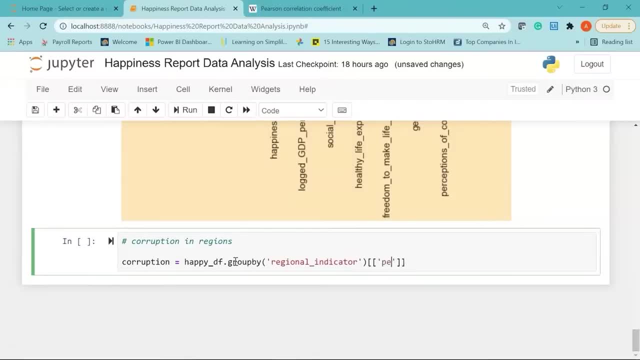 of the corruption, that is, perceptions of corruption. so I am going to pass in my variable name that is, perceptions of corruption, and I am going to use the mean function to find the average corruption in each of these regions. now let me just go ahead and print my 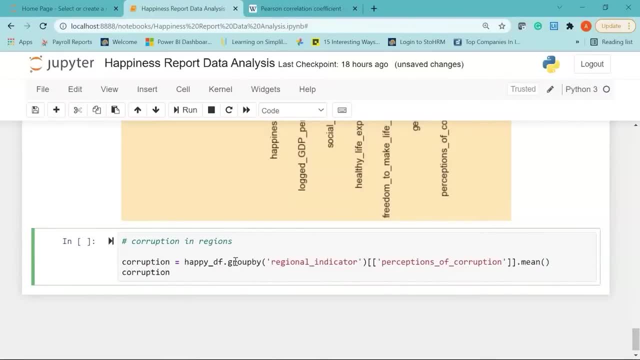 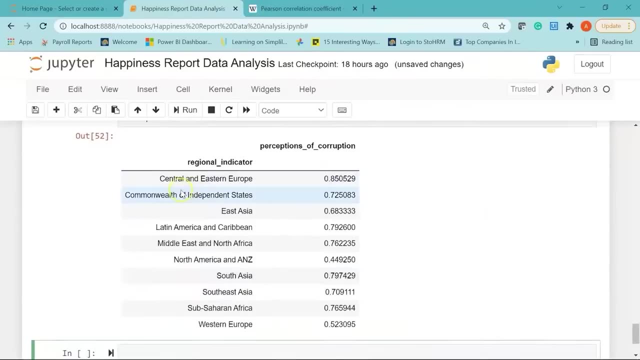 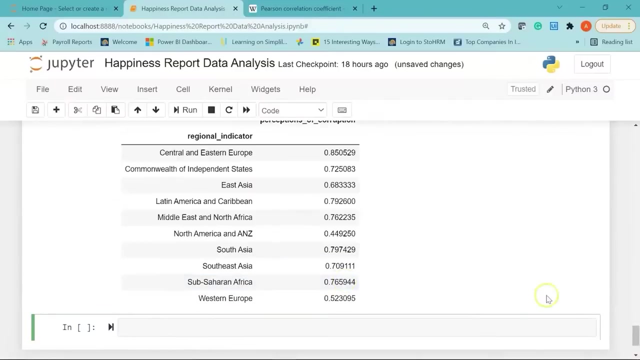 variable that is corruption. if I run it you can see here I have the values for the different regions and from here you can see that Central and Eastern Europe has the highest perceptions of corruption, as per the questions answered in the poll and if you see the table. 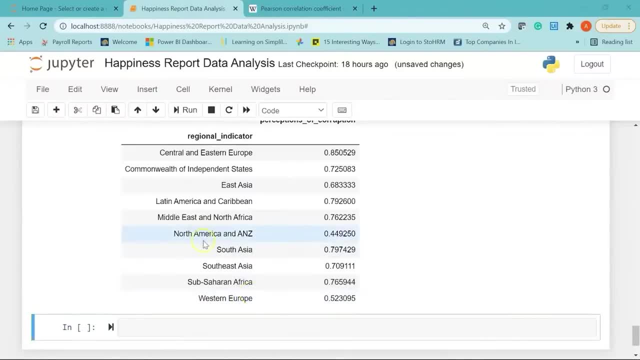 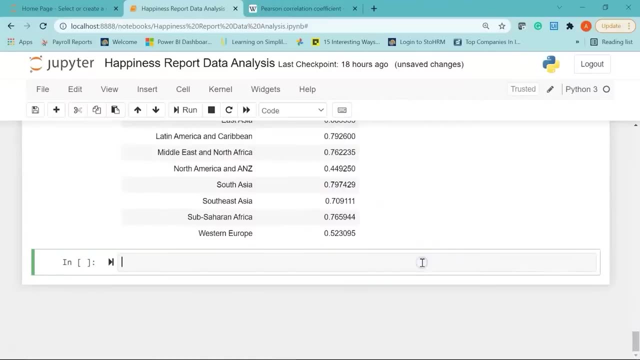 we have Western Europe and the North America region with the least perceptions of corruption. now we are going to visualize this using a bar plot now. so first of all, I will set my parameters by giving the figure size. I will say fig size, it's rather figure dot, fig size. 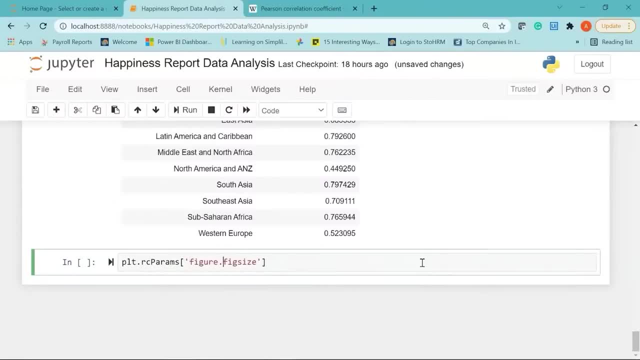 I will just add figure here. ok, and now let's say I will assign it as 12 comma 8. now I will give a title to my plot, so I will say plt, dot title, and my title of the plot is going to be perception of corruption. 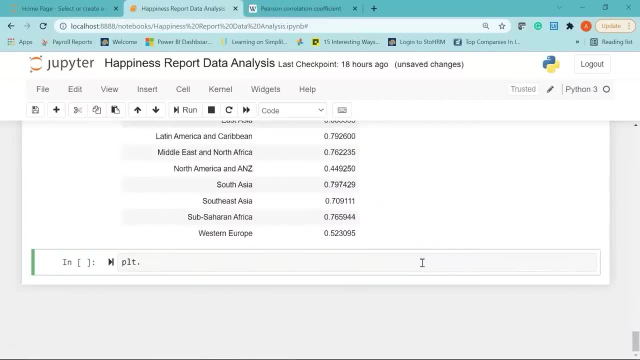 using a bar plot now. so first of all i will set my parameters by giving the figure size. i will say fig size, it's rather figure dot, fig size. i will just add figure here. ok, and now let's say i will assign it as 12 comma. 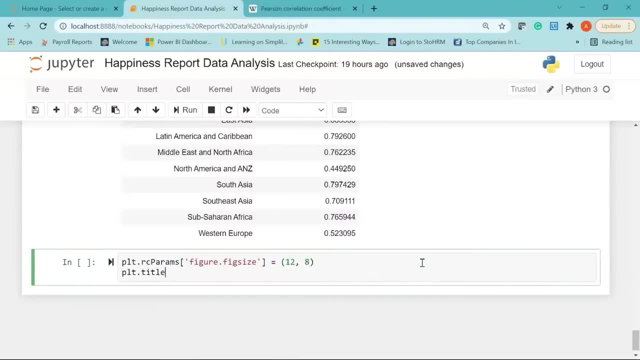 8. now i will give a title to my plot. so i will say plt dot title and my title of the plot is going to be perception of corruption in various regions. alright, then i am going to define my x label, so i will say x label will be: 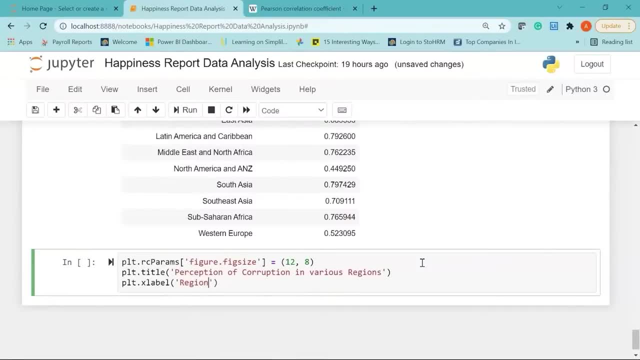 regions and we will set the font size of the x label to, let's say, 13, or let it be 15, and then we are going to set the y label. in y label i will have corruption index as the label name. again, we are going to set the font size. 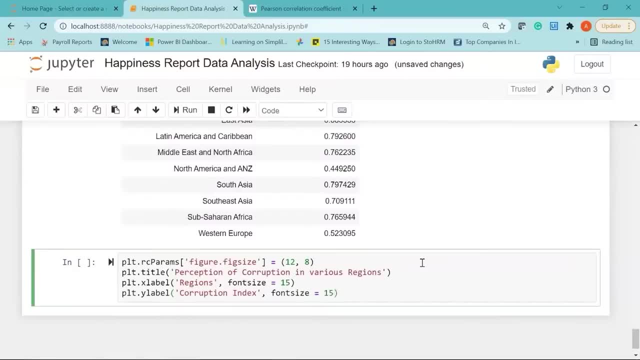 to 15. now i am going to use x ticks parameter, since i want to rotate the axis labels in the x axis by 30 degrees. so i will say rotation equal to 30 and i will say ha, which stands for horizontal alignment, equal to right. make sure this right should be within. 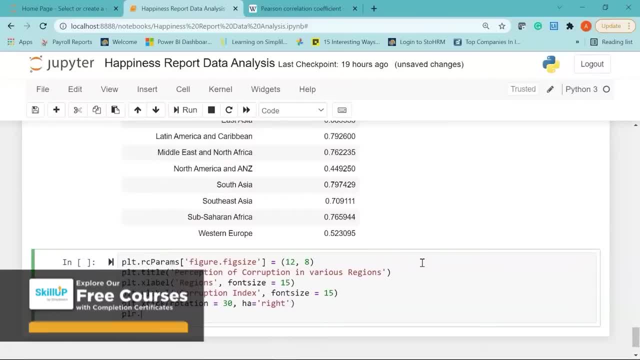 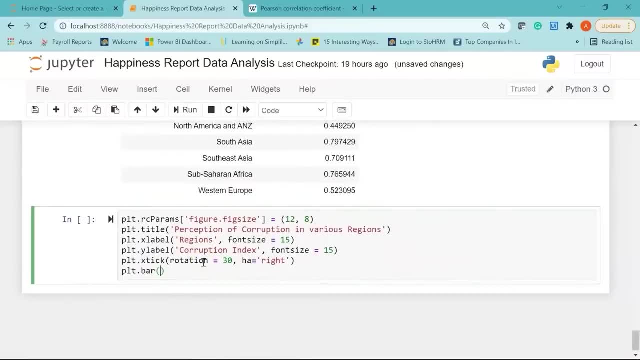 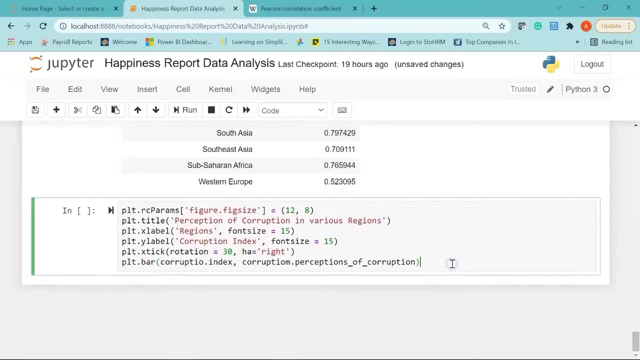 single quotes. and finally, i will say plt- dot- bar, because i am going to plot a bar graph. i will say corruption- dot- index comma. and then i will say corruption- dot- perceptions of corruption, which is my column name. alright, so i have my code ready for the bar plot. now let me just go ahead. 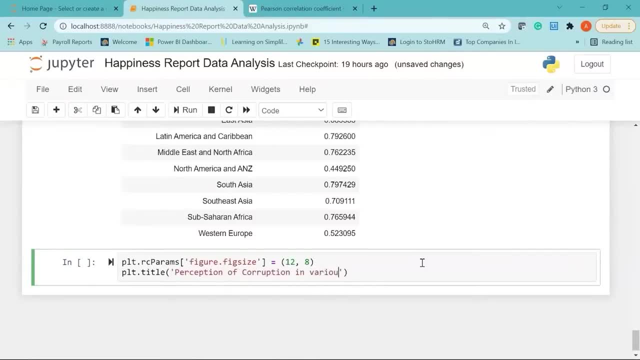 in various regions. alright, then I am going to define my x label. so I will say x label will be regions and we will set the font size of the x label to, let's say, 13 or let it be 15. then we are going to set the. 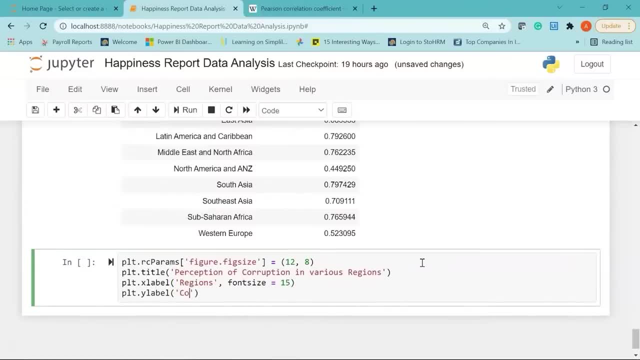 y label. in y label I will have corruption index as the label name. again, we are going to set the font size to 15. now I am going to use xtix parameter, since I want to rotate the axis labels in the x axis by 30 degrees. so I will say: 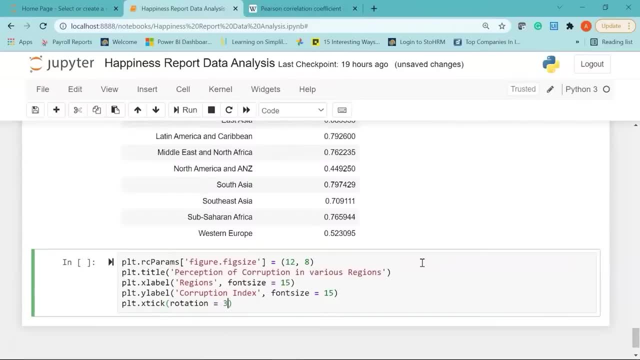 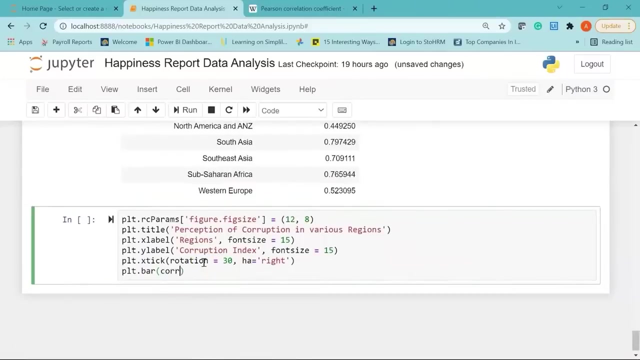 rotation equal to 30 and I will say ha, which stands for horizontal alignment, equal to right. make sure this right should be within single quotes. and finally, I will say plt, dot bar, because I am going to plot a bar graph. I will say corruption, dot index comma. 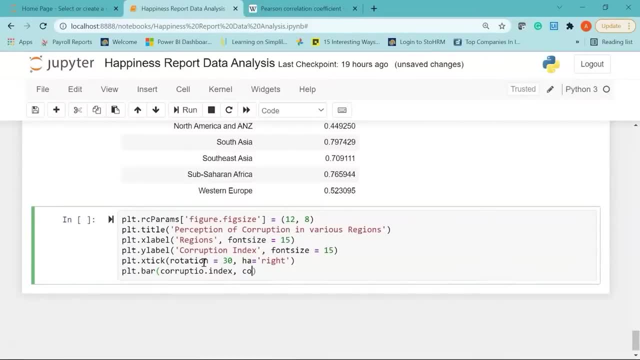 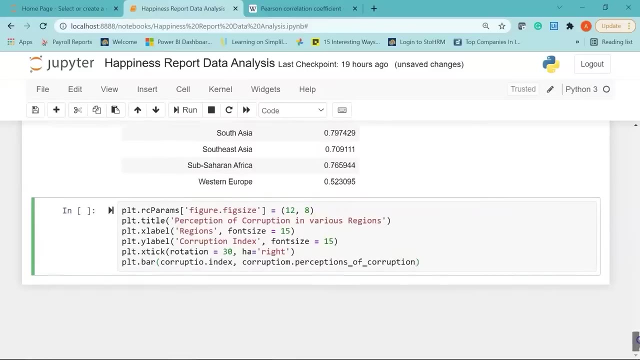 and then I will say corruption dot. perceptions of corruption, which is my column name. alright, so I have my code ready for the bar plot. now let me just go ahead and print the bar plot. make sure everything is correct. I will just hit shift, enter. ok, there is. 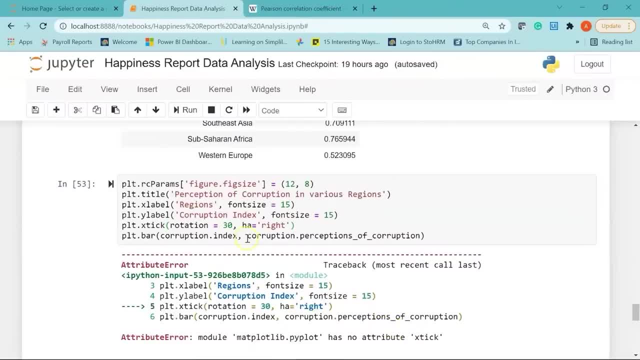 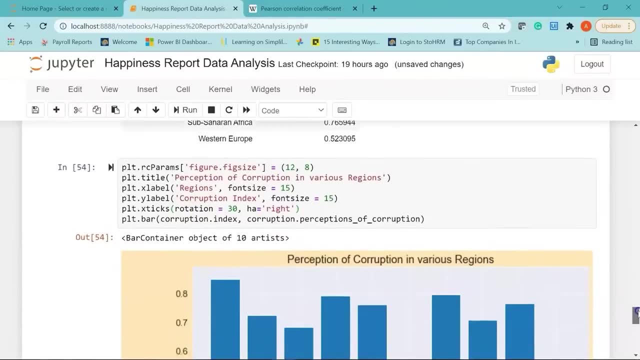 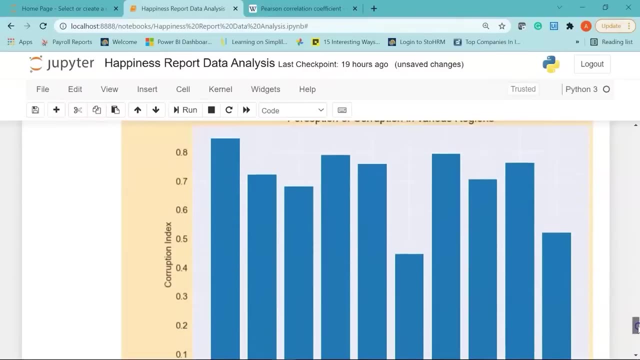 one mistake here. it says: ok, this should be xtix and not xtick. let me run it again. there you go. if I scroll down on the top, you have the title, which is perception of corruption in various regions. on the x axis you have the regions label. on the y axis you have the corruption index and if you see this, as per our table that we created, we have least corruption in North America and ANZ region, then we have the next least corruption in Western Europe, but we have the highest corruption in Central and Eastern Europe, as per 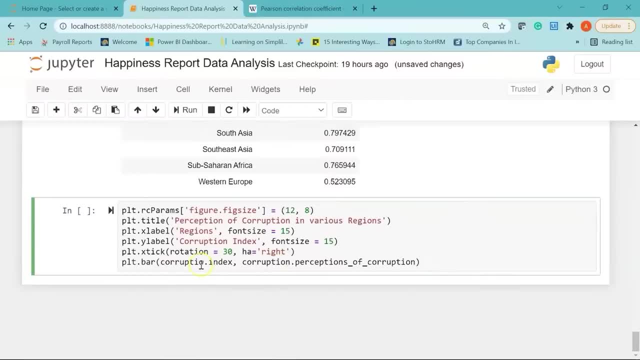 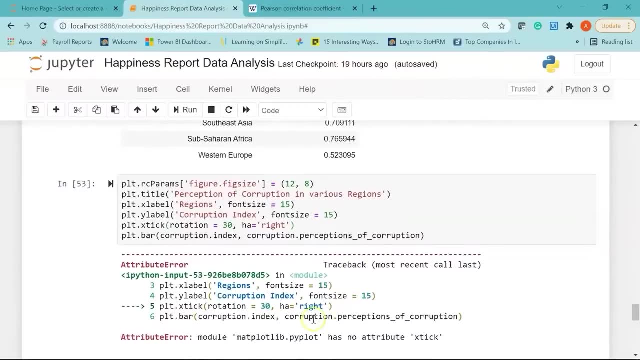 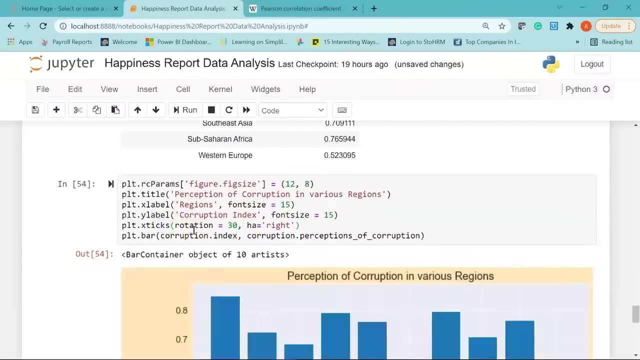 and print the bar plot. make sure everything is correct. i will just hit shift, enter- ok, there is one mistake here. it says ok, this should be x ticks and not x tick. let me run it again. there you go. if i scroll down on the top, you have the 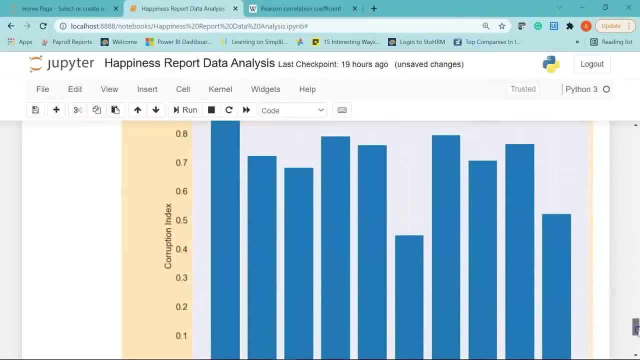 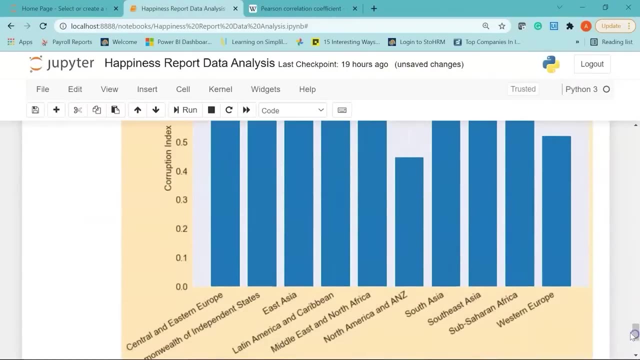 title, which is perception of corruption in various regions. on the x axis you have the regions label. on the y axis you have the corruption index and if you see this, as per our table that we created, we have least corruption in north america and ang region. then we have the next least corruption in western europe, but we have the highest corruption in central and eastern europe as per their citizens perception. similarly, we have the second and third highest corruption in latin america and caribbean, as well as south asia. cool. now, moving ahead, i am going to show you how you can find the. 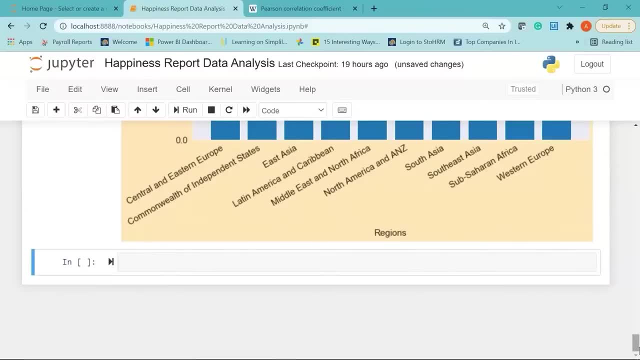 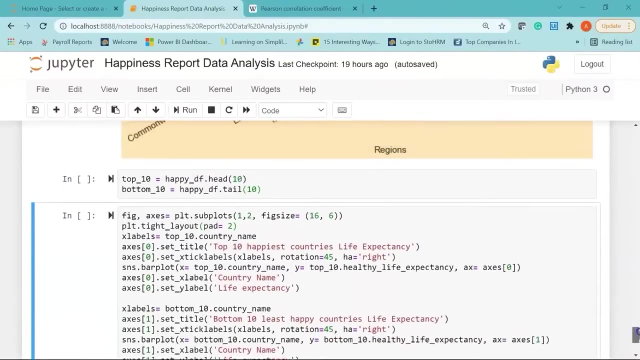 life expectancy of the top 10 happiest countries and bottom 10 happy countries. so for that, i am going to run you through the code and we will see the visualization side by side. ok, so i have my code written in these two cells. so first i am going to find out the 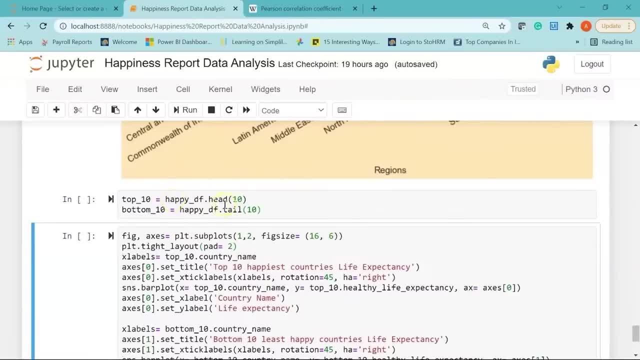 top 10 happiest countries and then i am going to find the bottom 10 happiest countries. so for that i am using the head function and i have passed in 10, since i want the top 10 country names and to get the bottom 10 countries as per their happiness score. 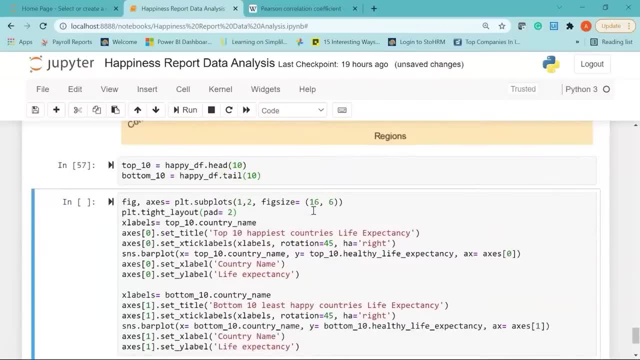 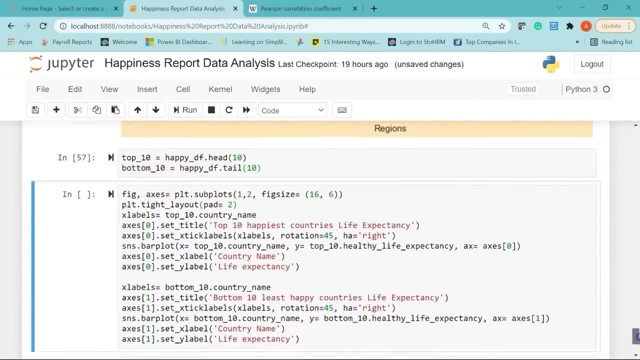 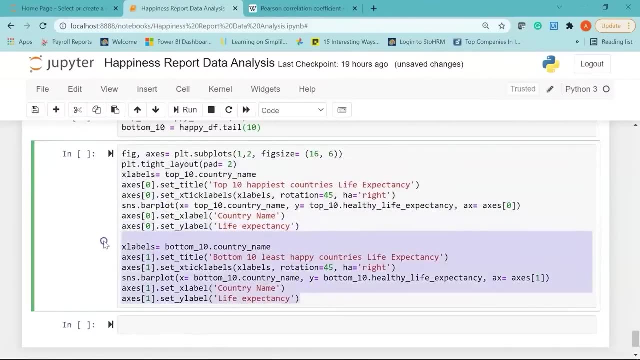 i am using the tail function, so let me just run it. so we have saved the result in two variables- top underscore 10 and bottom underscore 10- and to create the bar plots we are using two different codes. so here you can see i have set my. 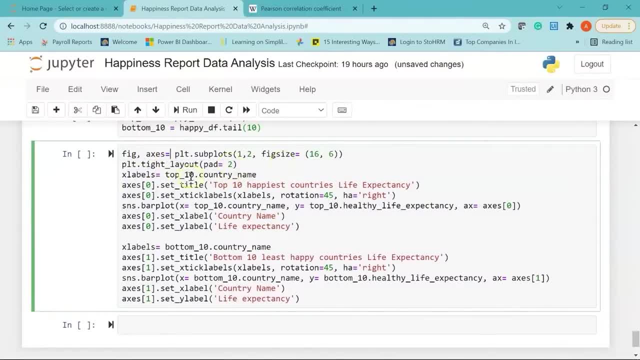 figure, size and axis, and then i have my x label as country name. after that i am setting my title of the bar plot to top 10 happiest countries. life expectancy. i have used my x tick label and i am rotating it by 45 degrees and i have my horizontal alignment. 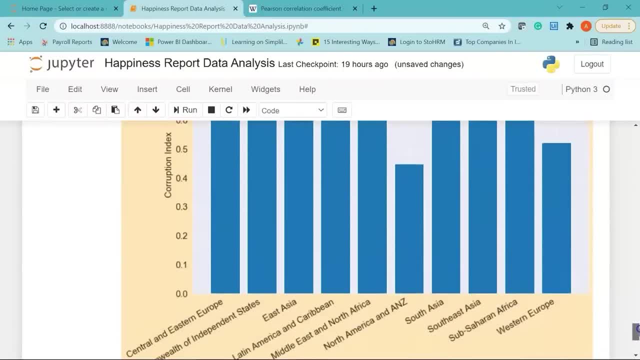 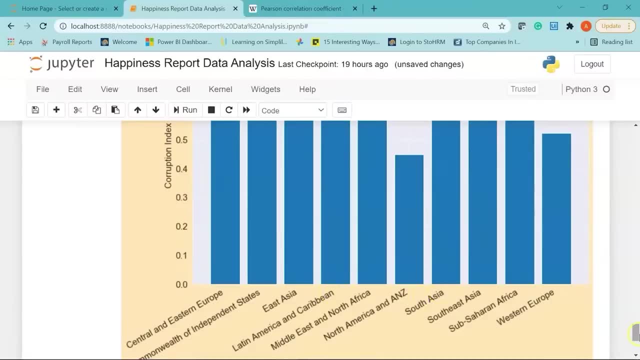 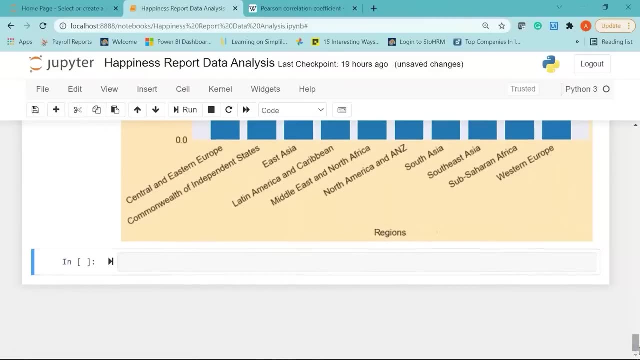 their citizens perception. similarly, we have the second and third highest corruption in Latin America and Caribbean, as well as South Asia. cool. now moving ahead, I am going to show you how you can find the life expectancy of the top 10 happiest countries and bottom 10 happy. 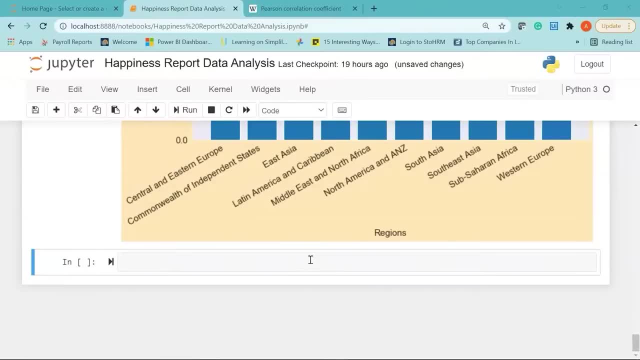 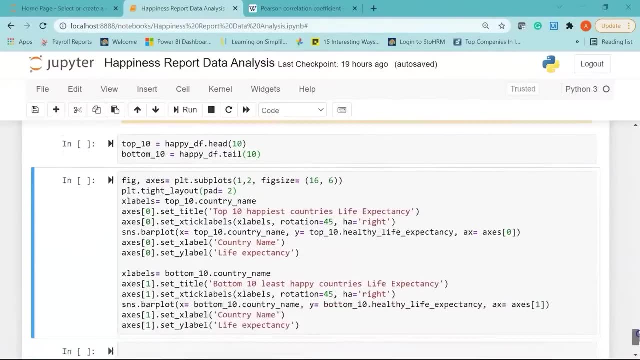 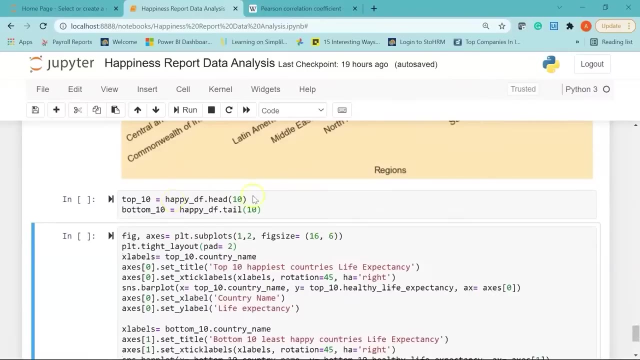 countries. so for that I am going to run you through the code and we will see the visualization side by side. ok, so I have my code written in these two cells. so first I am going to find out the top 10 happiest countries and then I am going to find the 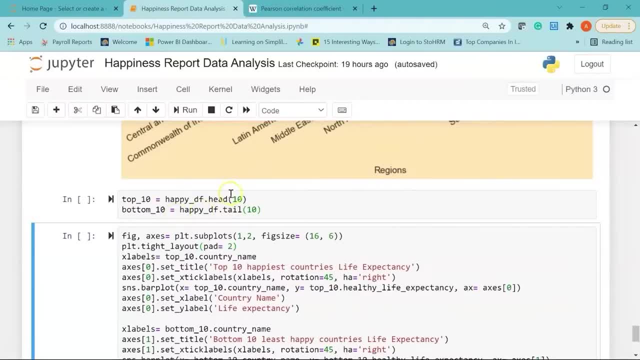 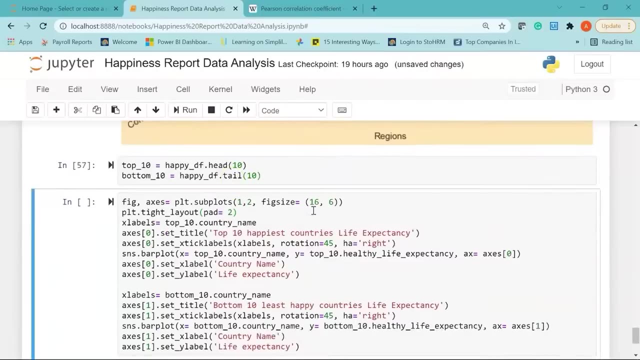 bottom 10 happiest countries. so for that I am using the head function and I have passed in 10. since I want the top 10 country names and to get the bottom 10 countries as per their happiness score, I am using the tail function. so let me just run it. 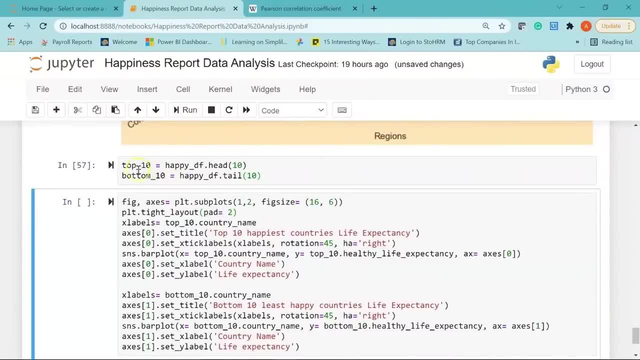 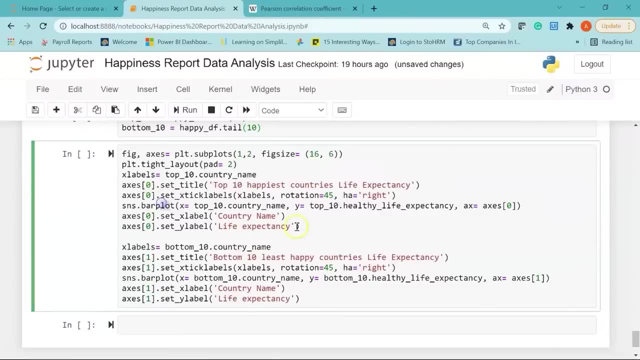 so we have saved the result in two variables- top underscore 10 and bottom underscore 10- and to create the bar plots we are using two different codes. so here you can see: I have set my figure size and axis, and then I have my x label as. 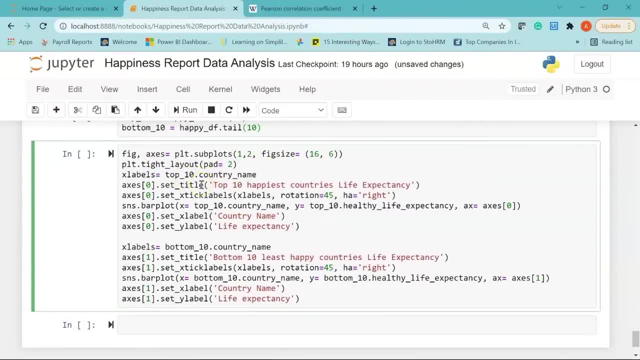 country name. after that I am setting my title of the bar plot to top 10 happiest countries. life expectancy. I have used my x tick labels and I am rotating it by 45 degrees and I have my horizontal alignment as right. you can see it here. we have used the bar plot function. 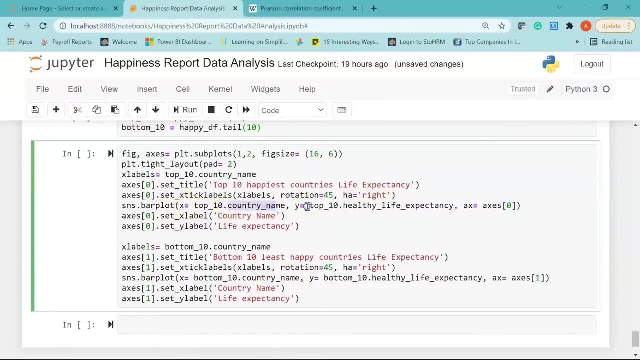 I have the x axis as country name and y axis as healthy life expectancy column and I have set my axis. then I am using the x labels and y labels as country name and life expectancy and similarly I have my bar plot for the bottom 10, least happy countries life expectancy. 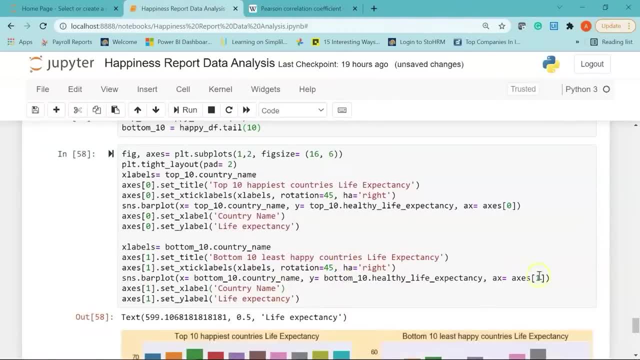 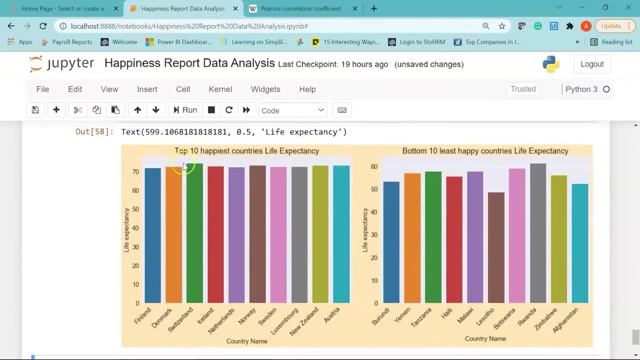 let's just run it and we will see the result. there you go now. if I scroll down, you can see we have two different bar plots. the first one is for the 10 happiest countries and then we have the bottom 10 least happy countries. so if you see, 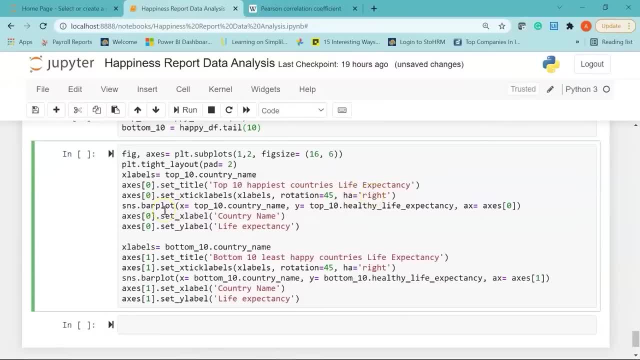 as right. you can see it here. we have used the bar plot function. i have the x axis as country name and y axis as healthy life expectancy column and i have set my axis. then i am using the x labels and y labels as country name and life expectancy and similarly. 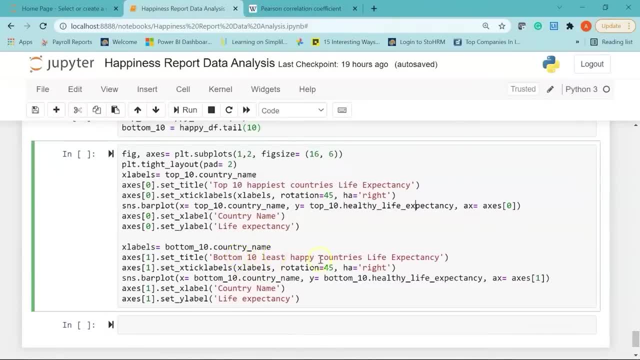 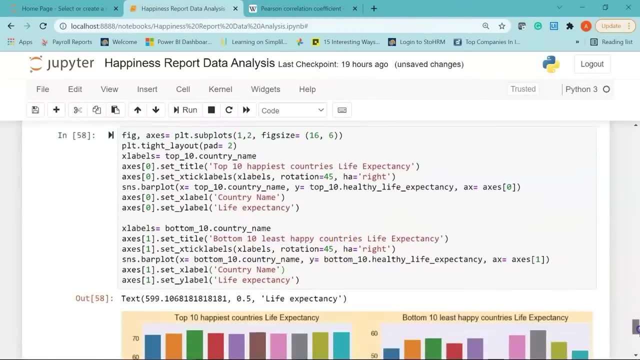 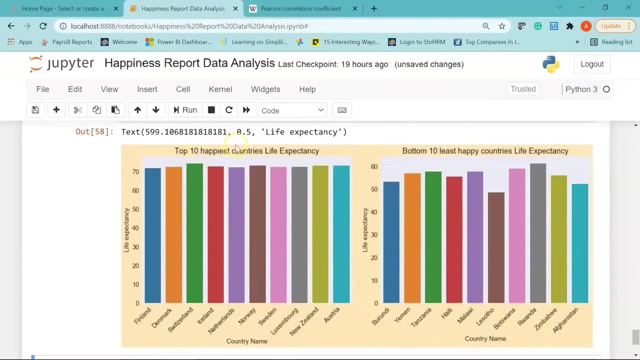 i have my bar plot for the bottom 10, least happy countries life expectancy. let's just run it and we will see the result. there you go. now, if i scroll down, you can see we have two different bar plots. the first one is for the 10 happiest. 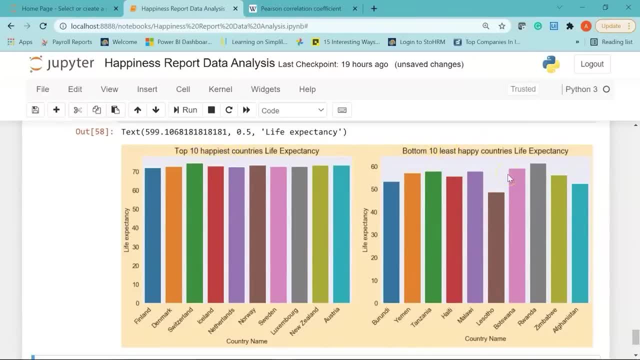 countries and then we have the bottom 10 least happy countries. so if you see, on an average, the top 10 happiest countries, life expectancy is above 70 years. so if you are from one of these countries, you are expected to live for more than 70 years. 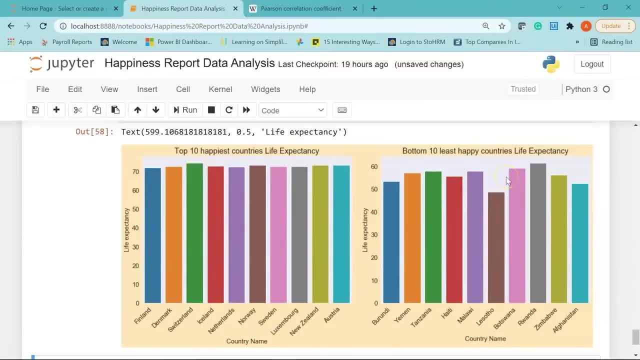 now, if you check the bottom 10 least happy countries, you see here lisotho has less than 50 life expectancy each and most of them are less than 60 years. so if you are from one of the top 10 happiest countries, you are expected to live. 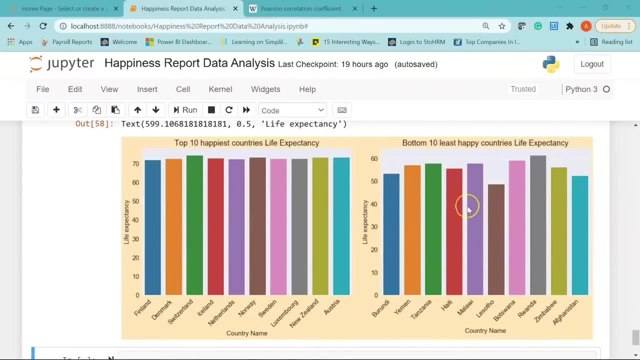 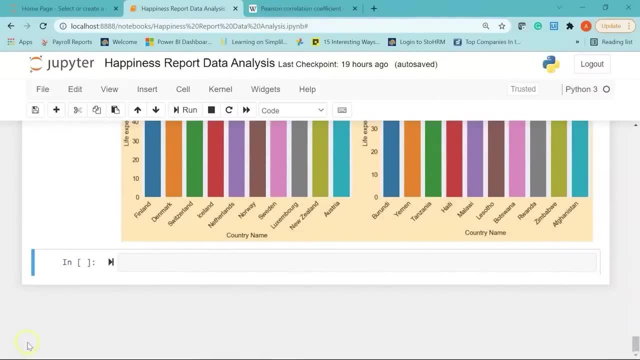 10 years more than these countries that lie in the bottom 10 region. cool, now moving ahead. alright. so now we are going to see the plot between freedom to make life choices and the happiness score. for this i am going to use a scatter plot, so i will first define my 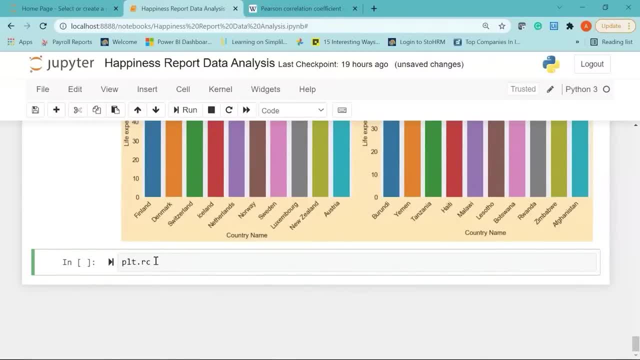 figure size. so i will say plt, dot, rc params, which stands for parameters. i am going to pass in my figure size, so i will say figure dot. fig size equal to, let's say, 15 comma 7. then, using the seaborn library and the scatter plot function, less than 50 life expectancy each, and most of them are less than 60 years. so if you are from one of the top 10 happiest countries, you are expected to live 10 years more than these countries that lie in the bottom 10 region. cool. 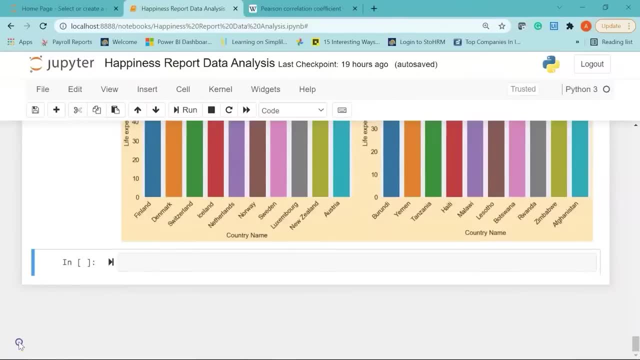 now moving ahead. all right. so now we are going to see the plot between freedom to make life choices and the happiness score. for this I am going to use a scatter plot, so I will first define my figure size. so I will say plt, dot, rc, params, which stands for parameters. 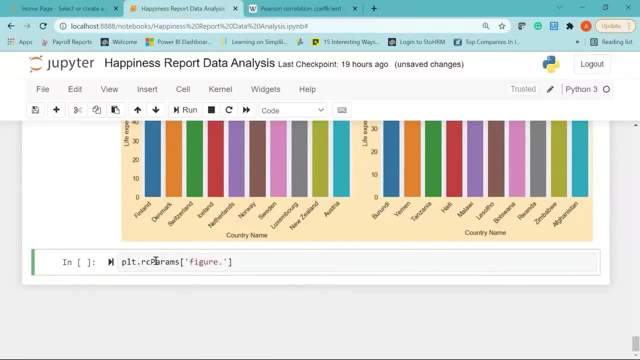 I am going to pass in my figure size, so I will say figure dot: fig size equal to, let's say, 15 comma 7. then, using the seaborn library and the scatter plot function, we will pass in the x axis. let's say the x axis is: 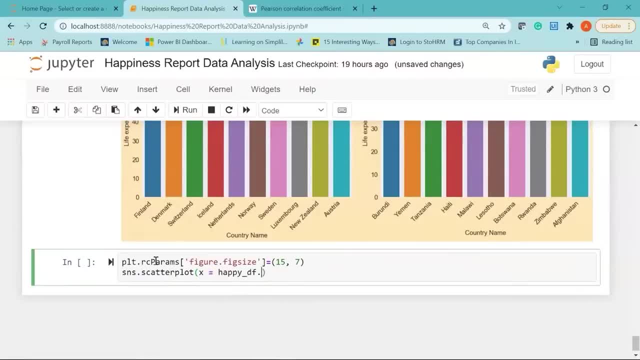 my data frame name, happy, underscore df, and I will have the freedom to make life choices in the x axis. so the column name is freedom, underscore. 2, underscore make, underscore- life and choices. I will give a comma and will pass in the y axis again. I am going to use my 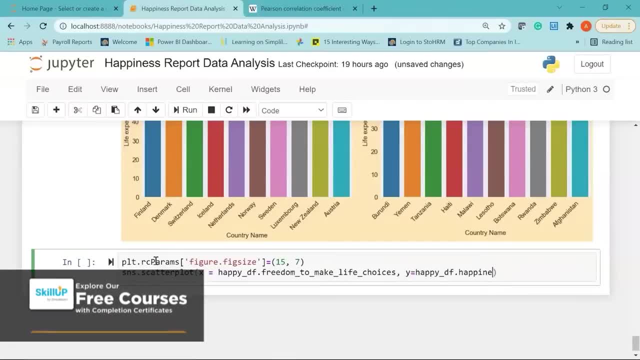 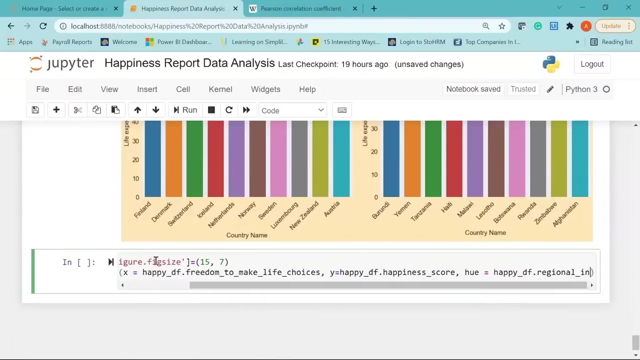 data frame name dot, and I will have the happiness score. I am also going to pass in a hue parameter to differentiate the different regions. so I will say df- dot- regional underscore indicator and I will give the size of the dots or the bubbles, as let's say. 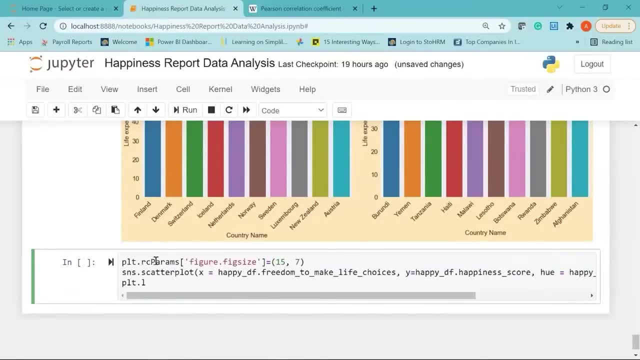 200. now I will say plt dot legend. I will place the legend at upper left corner, so I am giving the location, which is loc equal to upper left and font size let it be 12. I will say plt dot x label as freedom to make life. 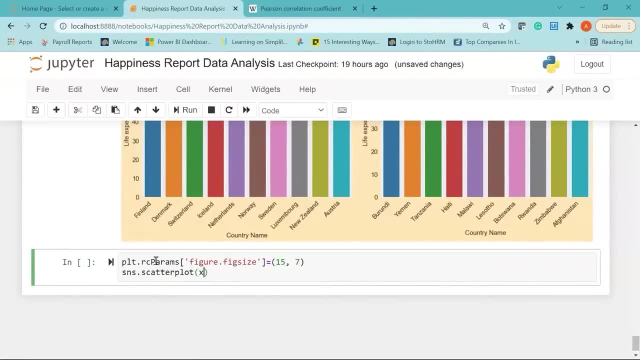 we will pass in the x axis. let's say the x axis is my data frame name happy, underscore df, and i will have the freedom to make life choices in the x axis. so the column name is freedom, underscore 2, underscore make, underscore life and choices. i will give a comma and will 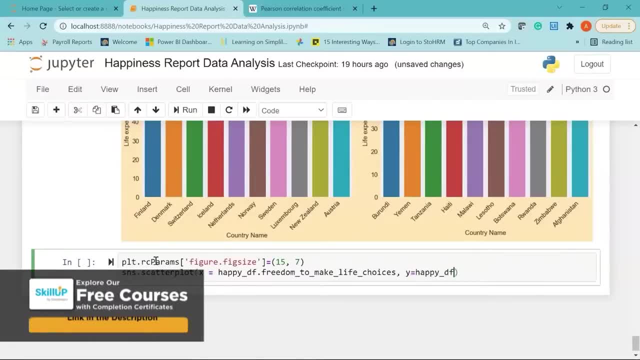 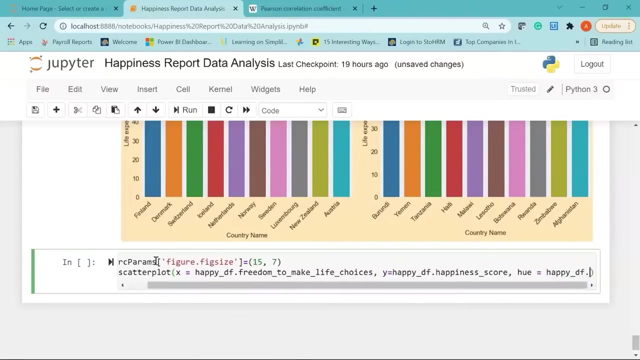 pass in the y axis again. i am going to use my data frame name, dot, and i will have the happiness score. i am also going to pass in a hue parameter to differentiate the different regions. so i will say df, dot- regional underscore indicator, and i will give the size. 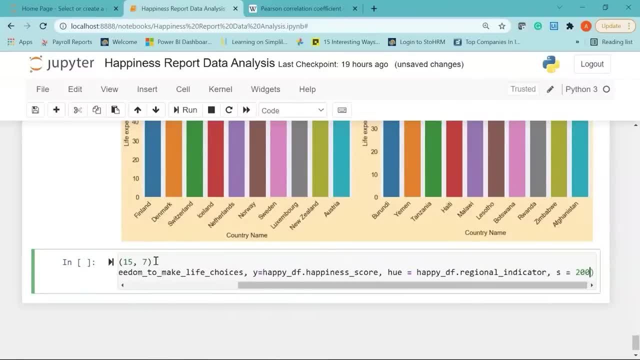 of the dots or the variables, as let's say, 200. now i will say plt dot legend. i will place the legend at upper left corner, so i am giving the location which is loc equal to upper left and font size. let it be 12. i will say: 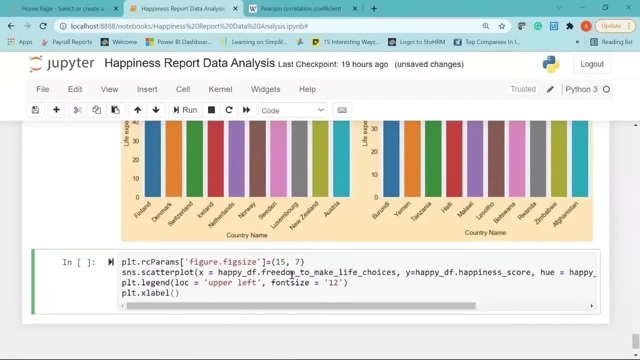 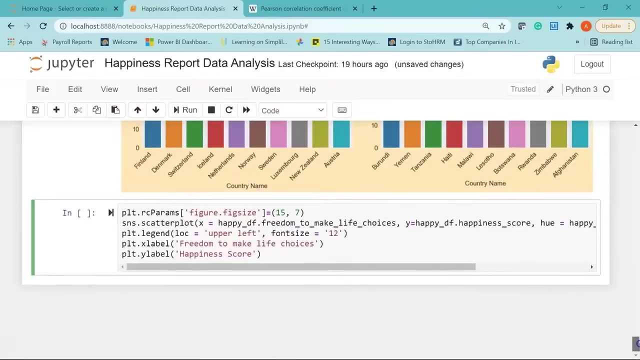 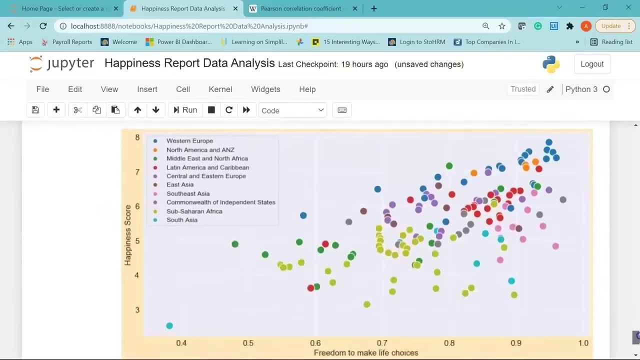 plt dot x label as freedom to make life choices, and my y label would be happiness score. alright, now we have the code written for the scatter plot that i want to create. let me just run it. there you go. so here we have the legend for the different. 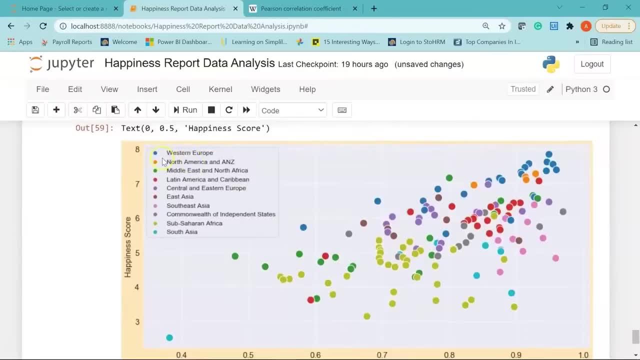 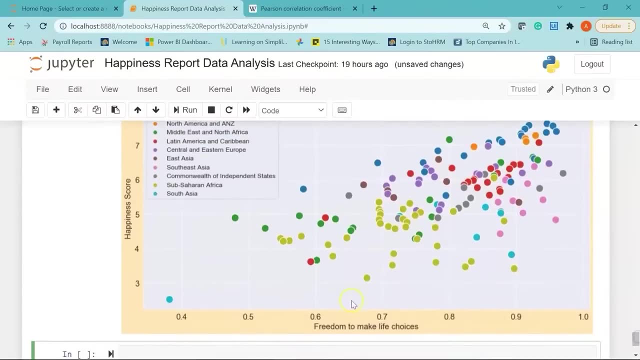 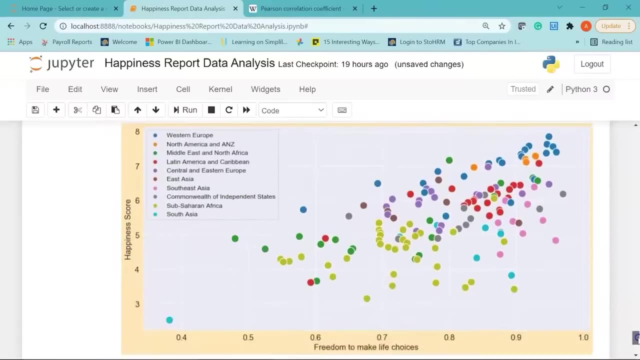 regions and we have the different colors for each of these regions and you can see here i have on the x axis, freedom to make life choices, and on the y axis we have the happiness score. so you can see it very clearly for the countries that lie in the 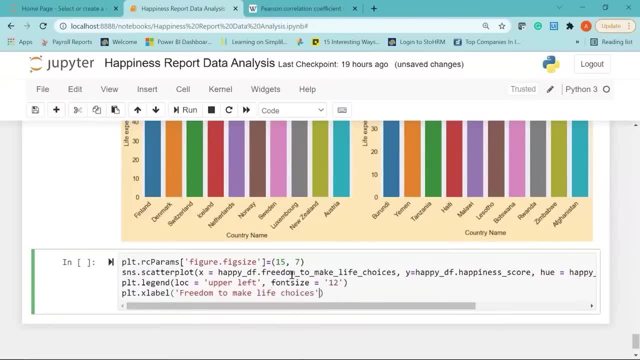 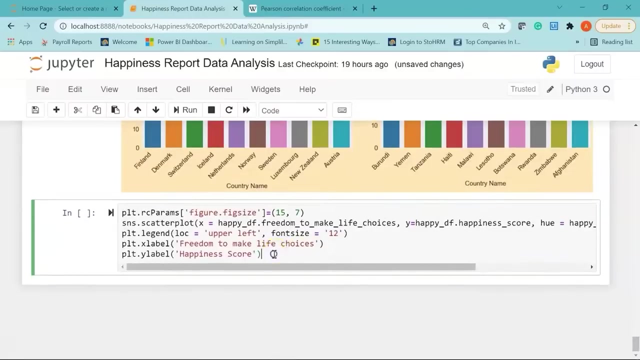 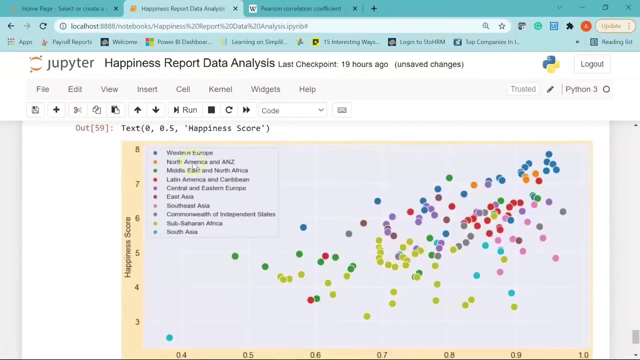 choices, and my y label would be happiness score. alright, now we have the code written for the scatter plot that I want to create. let me just run it there you go. so here we have the legend for the different regions and we have the different colors for each of these regions. 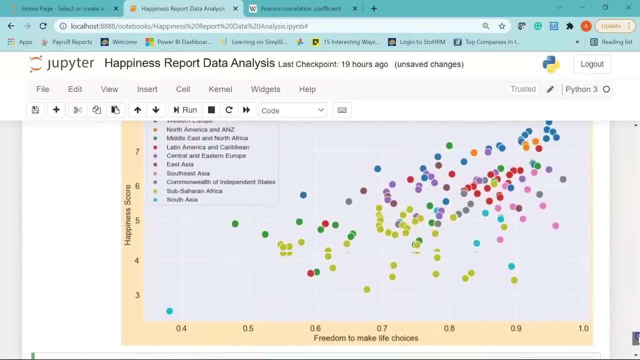 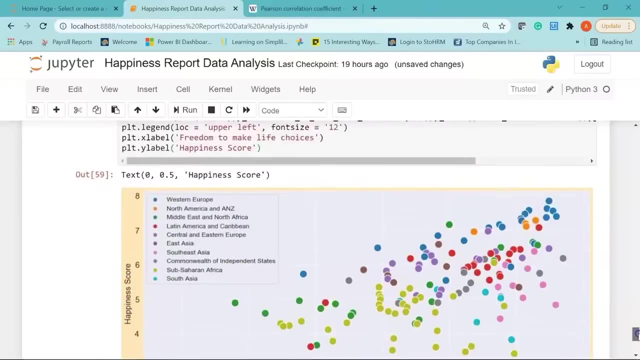 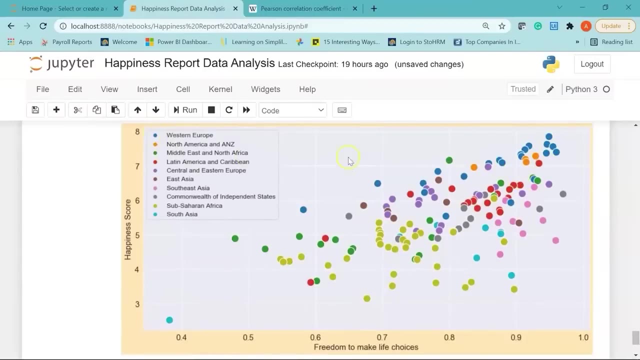 and you can see here I have on the x axis freedom to make life choices and on the y axis we have the happiness score. so you can see it very clearly. for the countries that lie in the western europe region, the blue dots, the freedom to make life choices is 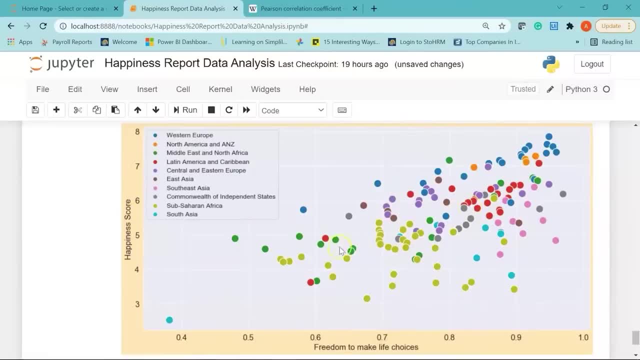 more, and so is the happiness score. then, if you see the values in the green region, which is for middle east and north africa, the freedom to make life choices is lower and hence the happiness score is also low. and for all these countries that are part of the sub saharan africa, 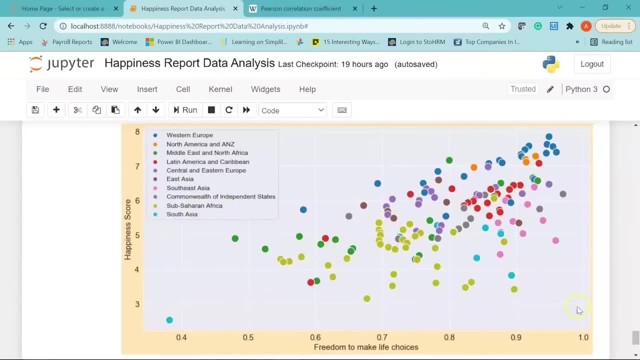 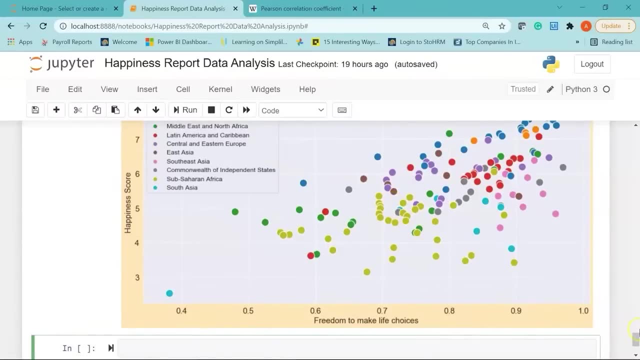 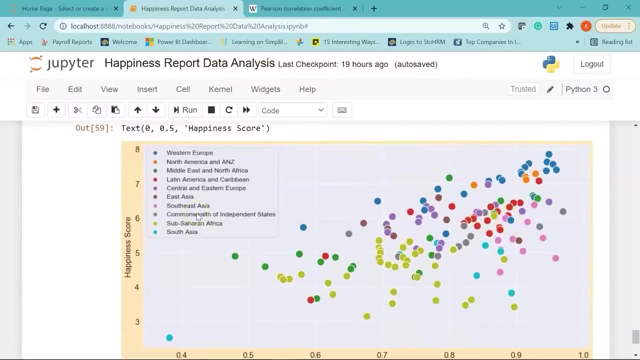 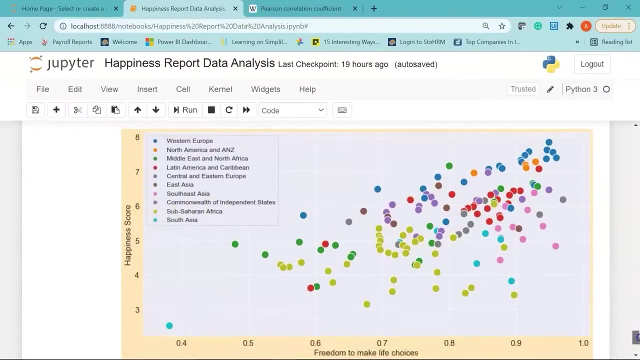 some of them have decent score for freedom to make life choices, but the happiness score is low. again now, if you focus on the pink dots, which is for the south east asian countries, the happiness score is comparatively lower, but the freedom to make life choices is more than. 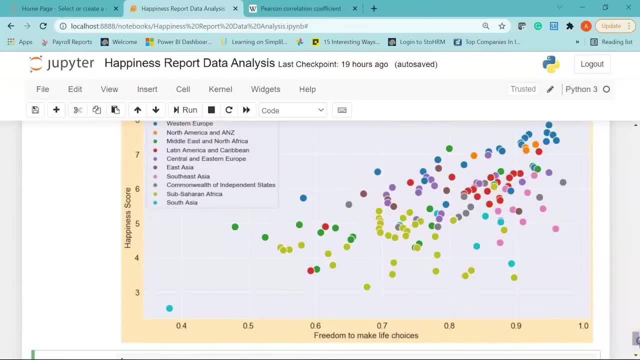 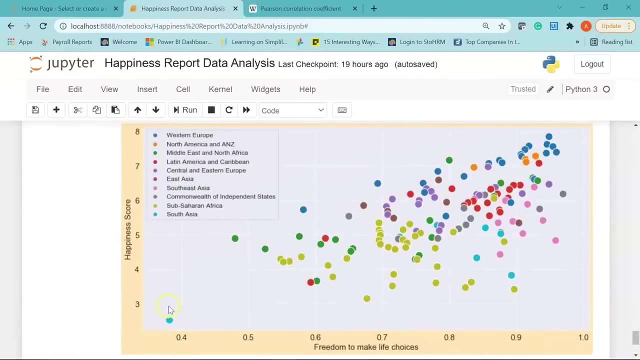 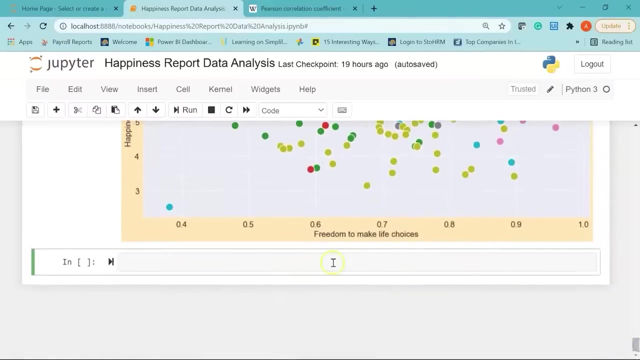 0.8- cool. and again we have one data point which is lying at the bottom. we can assume this is afghanistan. so in afghanistan, the freedom to make life choices is very low and even the happiness score is really low- cool. now moving to our next. 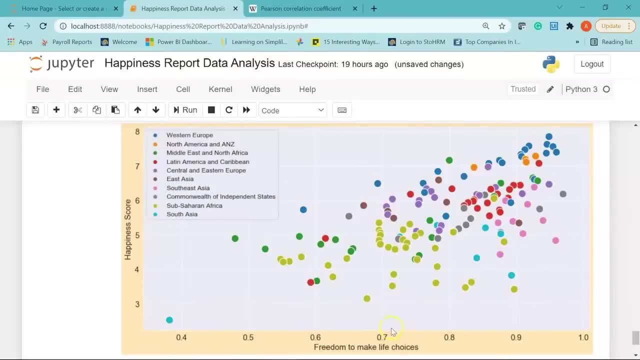 western europe region, the blue dots. the freedom to make life choices is more, and so is the happiness score. then, if you see the values, the green region, which is for middle east and north africa, the freedom to make life choices is lower and hence the happiness score is also low. and for 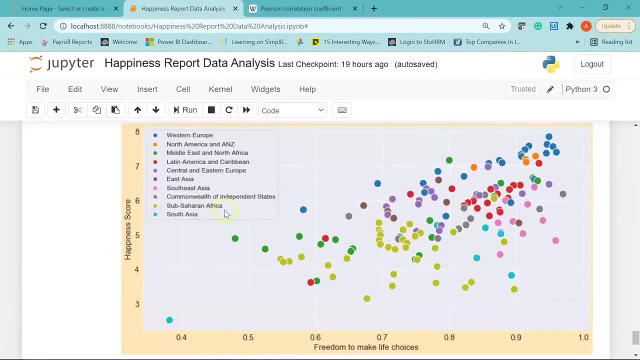 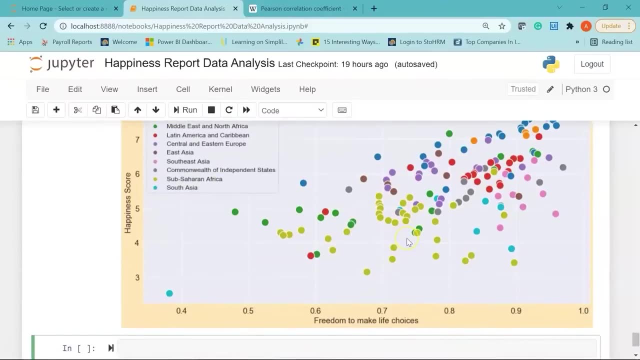 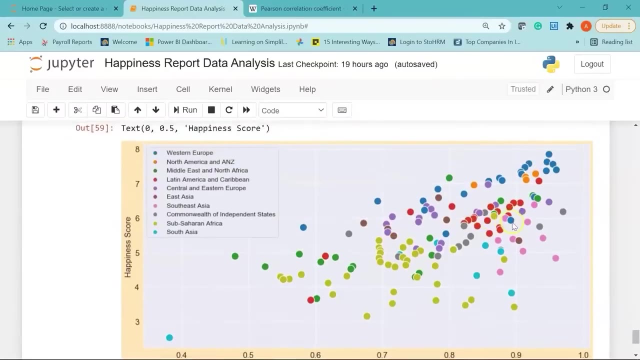 all these countries that are part of the sub saharan africa. some of them have decent score for freedom to make life choices, but the happiness score is low. again now if you focus on the pink dots, which is for the south east asian countries, the happiness score 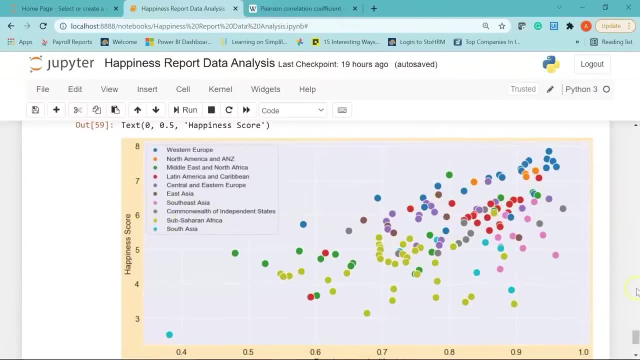 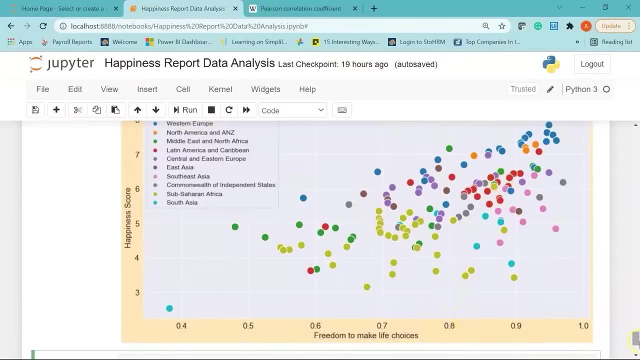 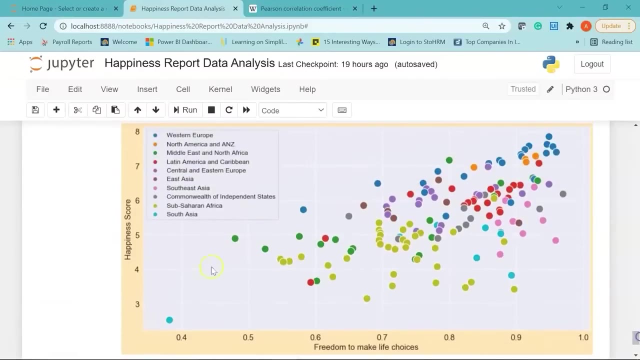 is comparatively lower, but the freedom to make life choices is more than 0.8. cool, and again we have one data point which is lying at the bottom. we can assume this is afghanistan. so in afghanistan, the freedom to make life choices is. 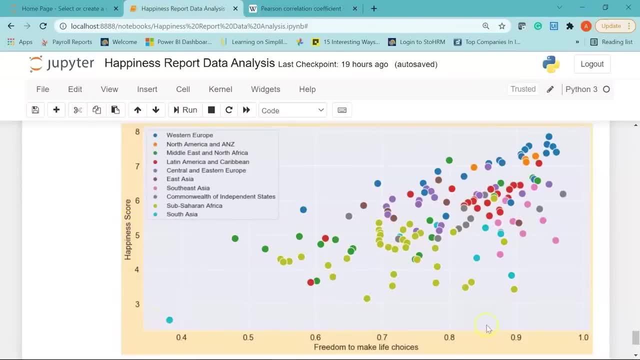 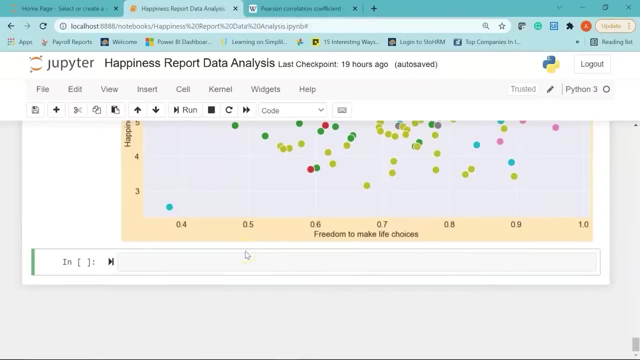 very low, and even the happiness score is really low- cool. now, moving to our next analysis, we are going to see the top 10 most corrupt countries. so first i am going to sort the perceptions of corruption column and find out the top 10 countries in the list. 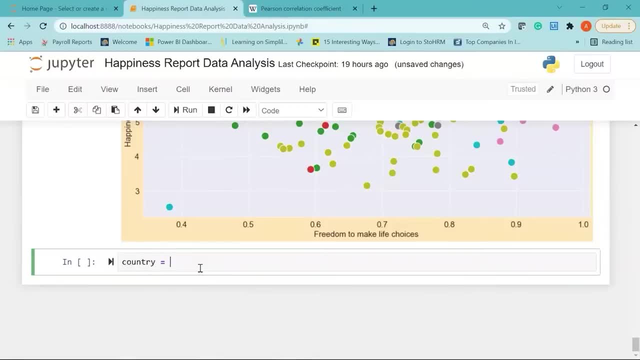 so for that i am going to create a variable called country. i will have my data frame name, that is happy. underscore df, dot. sort underscore values by. i am going to sort by column, that is, perceptions of corruption, dot head, and i want to find the top 10 most corrupt countries. 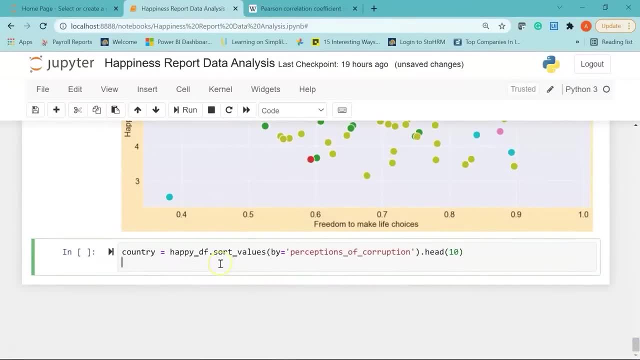 as per the poll. and then i am going to pass in the figure size, so i will say plt dot rc params. and then i am going to set the figure size, so i will say figure dot- fig size. make sure there is no spelling mistake. let's say the. 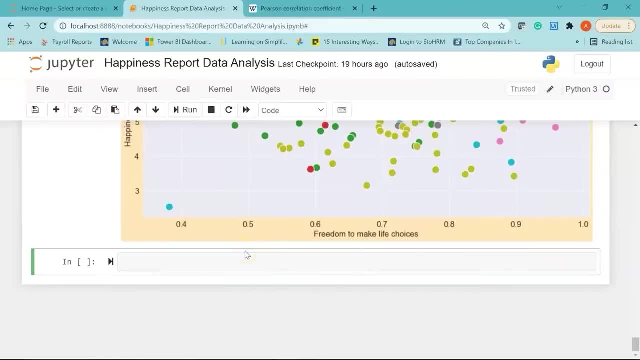 analysis we are going to see the top 10 most corrupt countries. so first i am going to sort the perceptions of corruption column and find out the top 10 countries in the list. so for that i am going to create a variable called country. i will have my data. 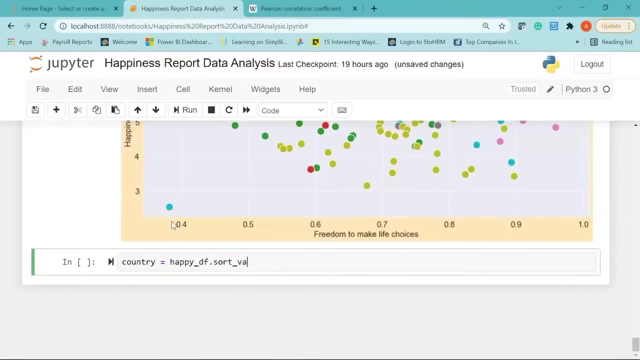 frame name, that is happy. underscore: df, dot. sort underscore values by: i am going to sort by column, that is, perceptions of corruption by dot head, and i want to find the top 10 most corrupt countries as per the poll, and then i am going to pass in the figure size. 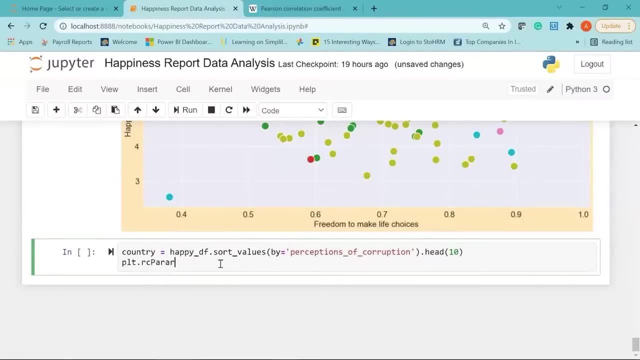 so i will say plt dot rc params, and then i am going to set the figure size. so i will say figure dot, fig size. make sure there is no spelling mistake. let's say the figure size is 12 comma 6. i will pass in the title. 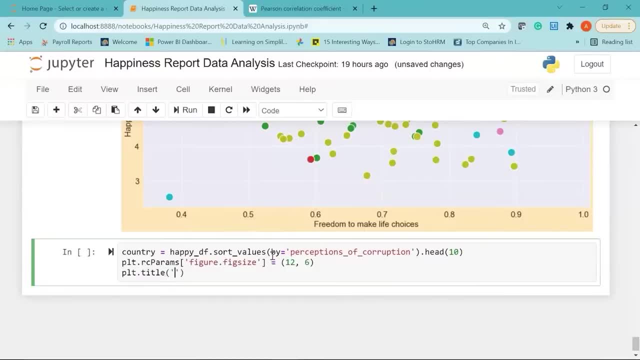 so i will say plt dot title. let's say the title of my plot is going to be countries with most corrupt perception of corruption. after that i will say plt dot x label. in the x label i will have country and i will set the font size to. 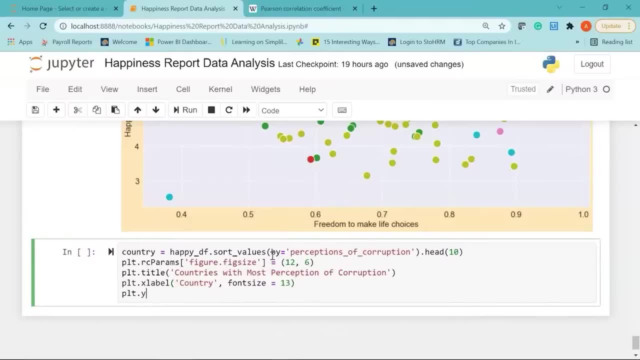 13. then i will say plt dot y label- y label. i will have the corruption index. next i will pass in the font size for the y label. again, it is going to be 13. now i will say plt dot x ticks. i am going to rotate it. 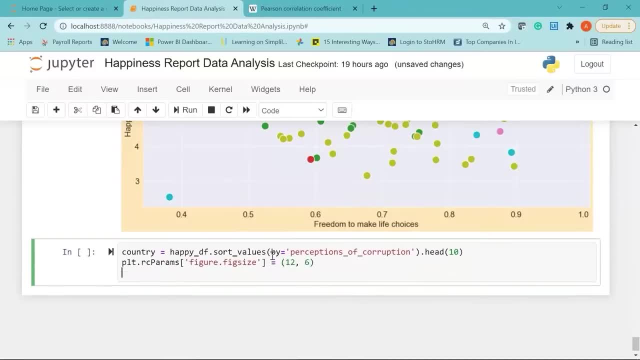 figure size is 12 comma 6. i will pass in the title. so i will say plt- dot title. let's say the title of my plot is going to be countries with most perception of corruption. after that i will say plt- dot x label in the x label. 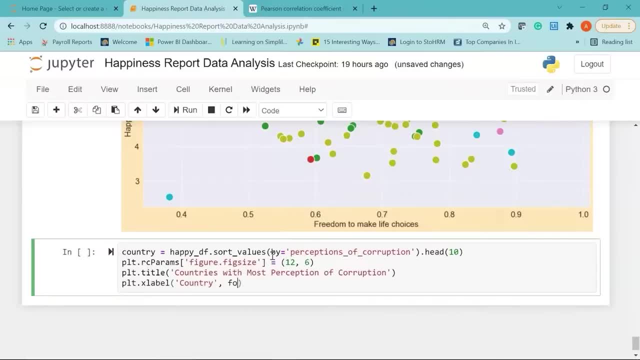 i will have country and i will set the font size to 13. then i will say plt, dot y label. in y label i will have the corruption index. next i will pass in the font size for the y label. again, it is going to be 13. 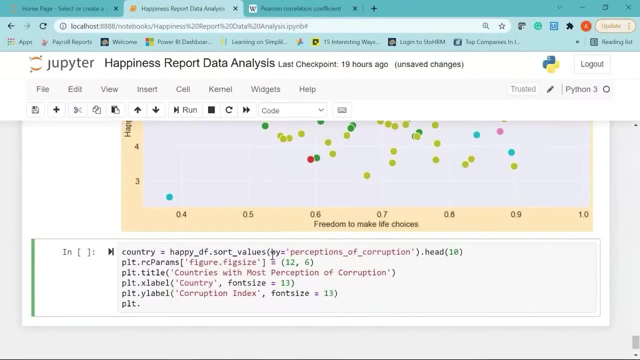 now i will say plt, dot x ticks. i am going to rotate it by 30 and i will say horizontal alignment equal to right. then i will have my bar function or the bar plot function. so i will say plt, dot bar. i am going to pass in country dot. 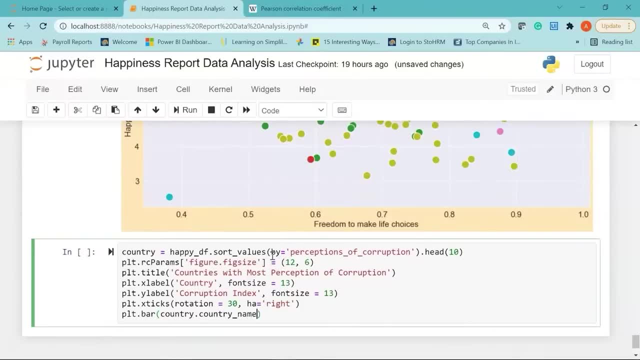 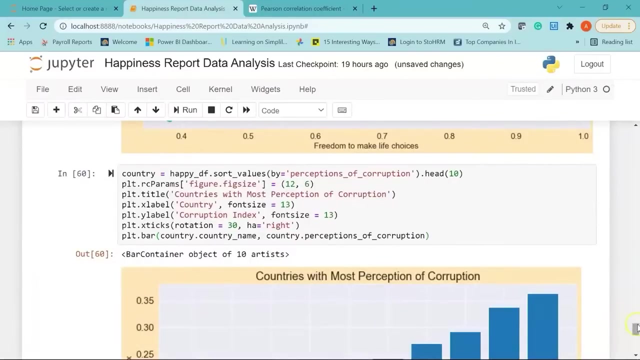 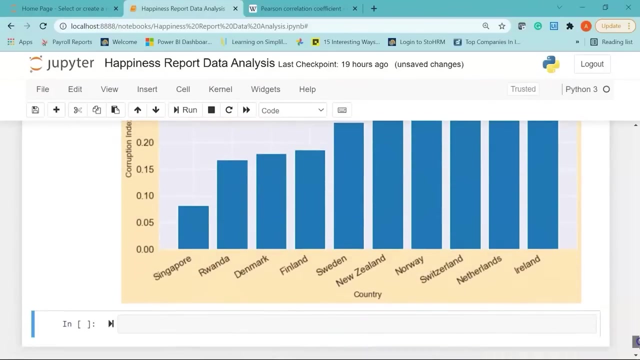 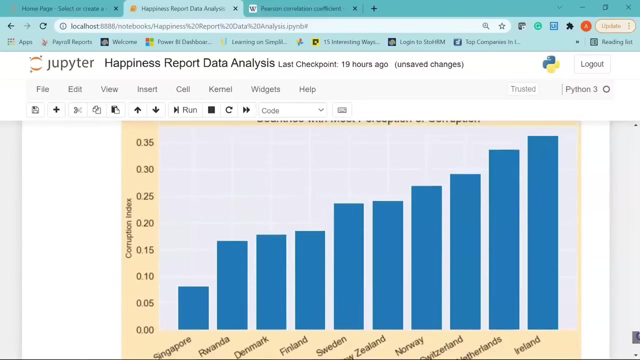 country underscore name and then we will have my variable country dot the column name. that is perceptions of corruption. alright, now, if i run it, you can see here. so these are the countries with the least perceptions of corruption. so singapore has the lowest corruption index, and then we have 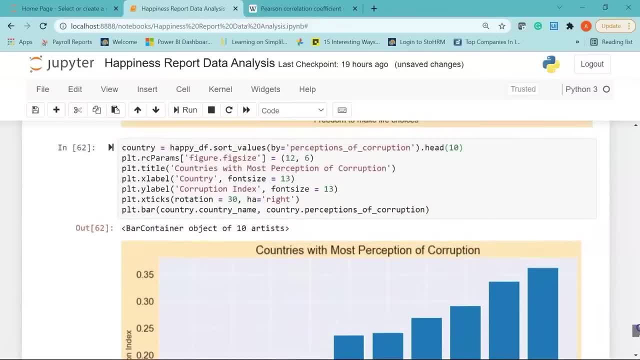 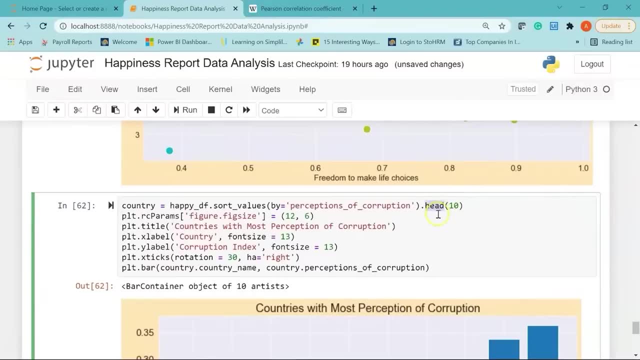 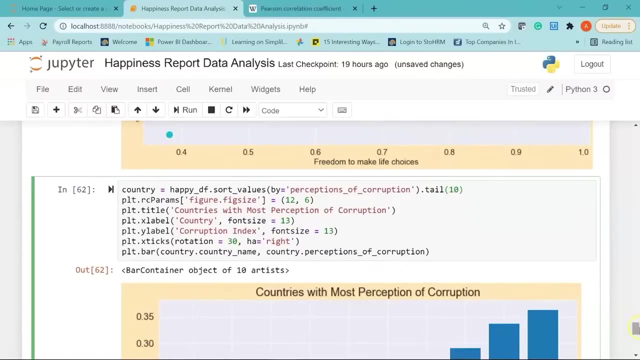 rwanda, denmark, finland. now, if you want to see the countries with the highest perceptions of corruption, you need to change this head to tail of 10, since we are sorting it in ascending order, so we would want to know the bottom 10 countries. if i run it, there you go. so these are the countries with the most perception of corruption. you have slovakia, lisoto, kosovo, there is ukraine, afghanistan, bulgaria, romania and croatia. all of these countries have a corruption index of more than 0.85. 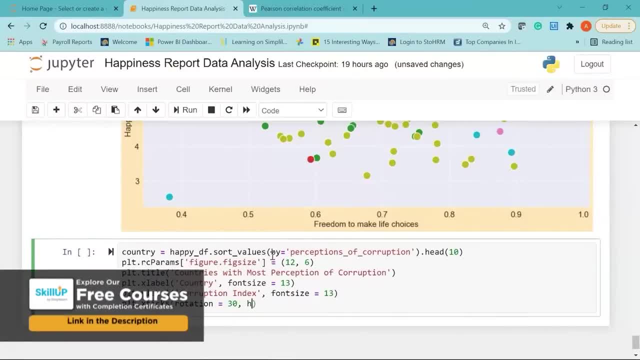 by 30 and i will say horizontal alignment equal to right. then i will have my bar function or the bar plot function. so i will say plt, dot bar. i am going to pass in country dot, country, country underscore name and then we will have a variable country. 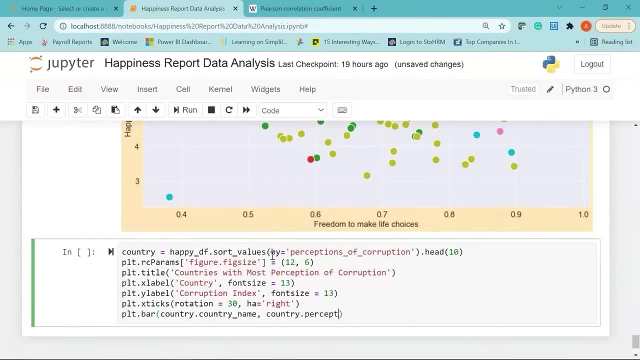 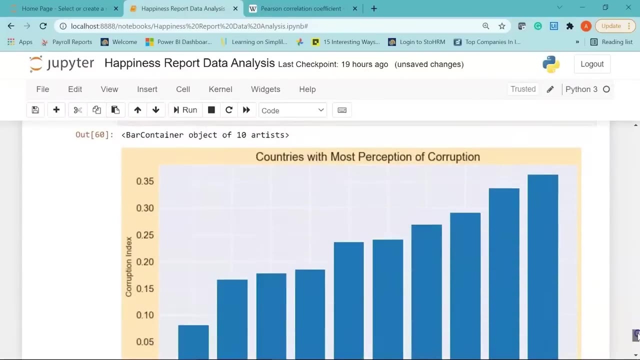 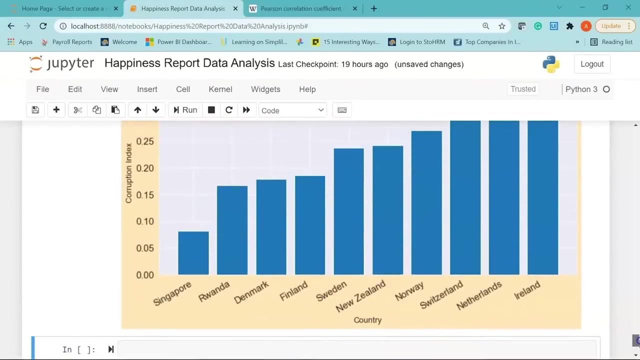 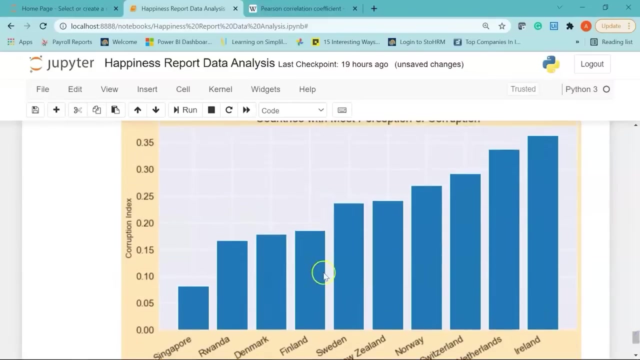 dot the column name, that is perceptions of corruption. all right now, if i run it, you can see here. so these are the countries with the least perceptions of corruption. so singapore has the lowest corruption index, and then we have Rwanda, Denmark, Finland. now, if you want to, 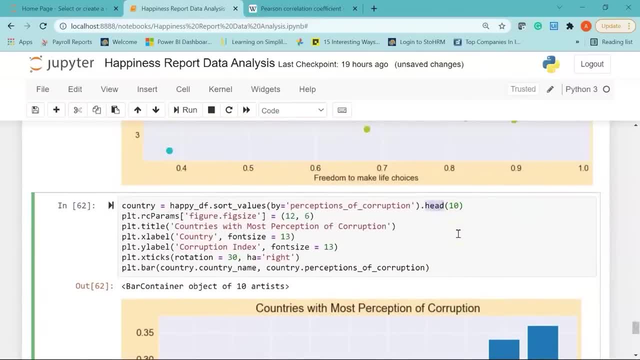 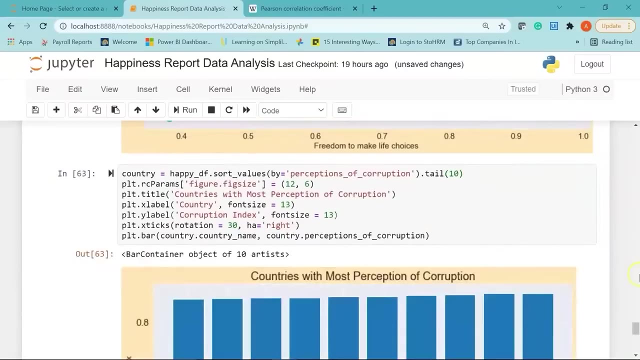 see the countries with the highest perceptions of corruption. you need to change this head to tail of 10, since we are sorting it in ascending order. so we would want to know the bottom 10 countries. if i run it, there you go. so these are the countries with the most. perception of corruption. you have slovakia, lisoto, kosovo, there is ukraine, afghanistan, bulgaria, romania and croatia. all of these countries have a corruption index of more than 0.85. cool, now, coming to the final section of this. 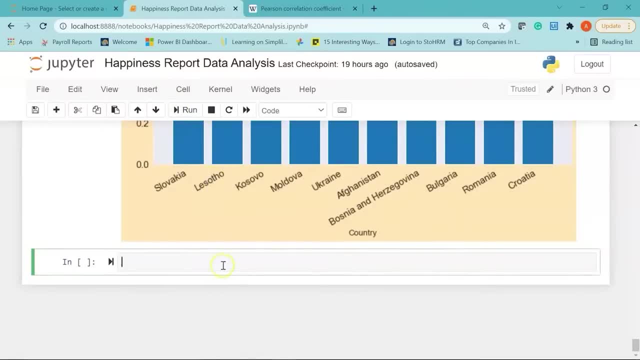 interesting video on happiness report: data analysis for 2021. i want to visualize a scatter plot that will tell us how the corruption varies in terms of happiness score. so i will just say a comment as corruption versus happiness. ok, so first of all, i will set my 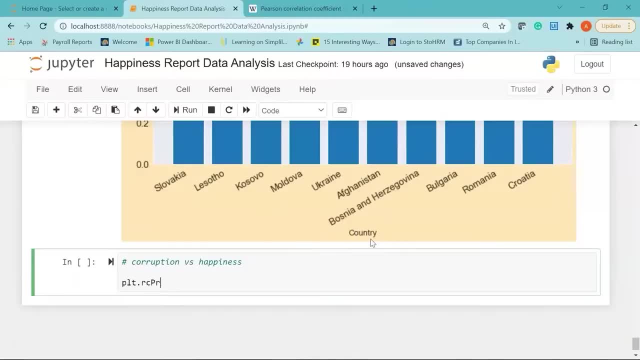 figure size. so i will say pltrc params within single quotes. i will give the figure size as 15 comma 7. then i am going to use the scatter plot function that is part of the seaborn library in the x axis. i will have my column that is. 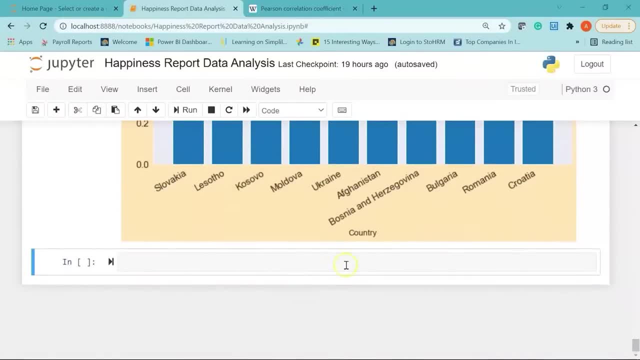 cool. now, coming to the final section of this interesting video on happiness report: data analysis for 2021, i want to analyze a scatter plot that will tell us how the corruption varies in terms of happiness score. so i will just say a comment as corruption vs happiness. 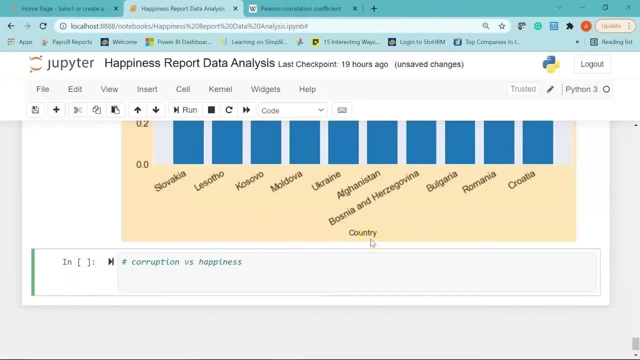 ok, so first of all i will set my figure size. so i will say plt, dot, rc params within single quotes. i will give the figure size as 15 comma 7. then i am going to use the scatter plot function that is part of the seaborn library. 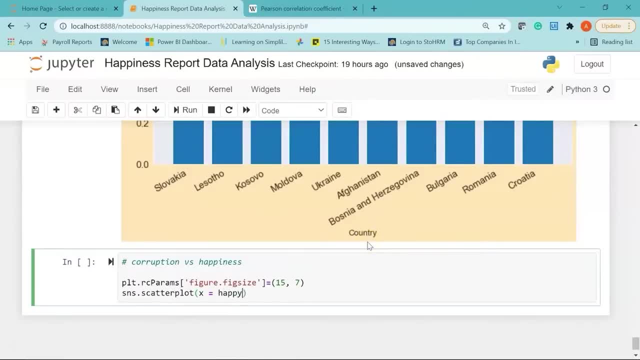 in the x axis i will have my column. that is corruption, or rather we will have the happiness score in the x axis. so i will say happy underscore: df, dot column name: that is happiness score. let me give a comma. and in the y axis we will have 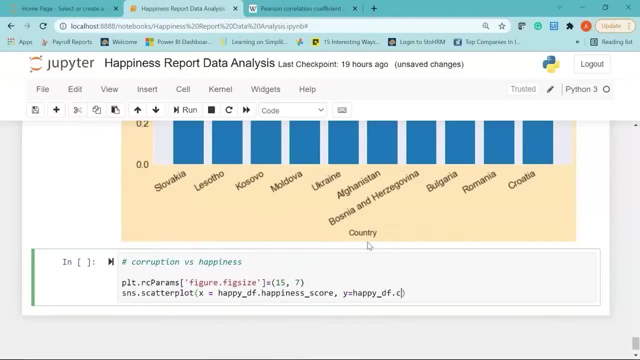 the corruption column. so i will say happy, underscore df, dot- perceptions of corruption. and then in hue we will have the region that is regional underscore indicator. so i will say happy, underscore df, dot, regional indicator. and i am going to give the size of the dots. so i will say: 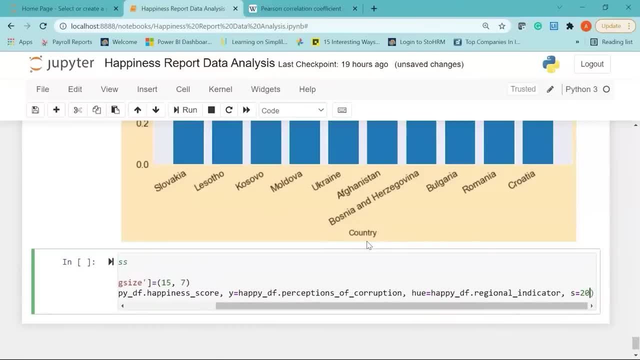 s equal to 200. then i am going to say plt dot legend. i am going to put it as at lower left corner this time, so i am giving my location as lower left and the font size of the legend i want is 14. after that i will just 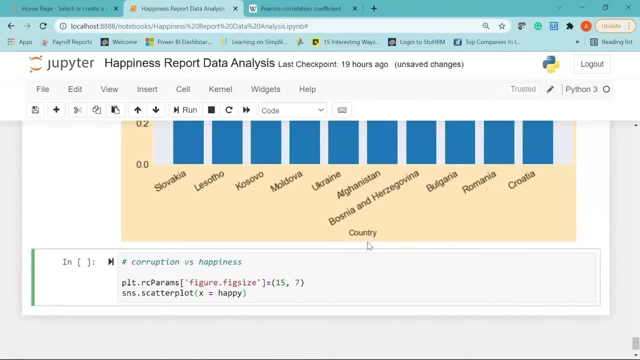 corruption. or rather we will have the happiness score in the x axis. so i will say: happy, underscore df, dot. column name: that is happiness score, let me give a comma. and in the y axis we will have the corruption column. so i will say happy, underscore, df, dot. 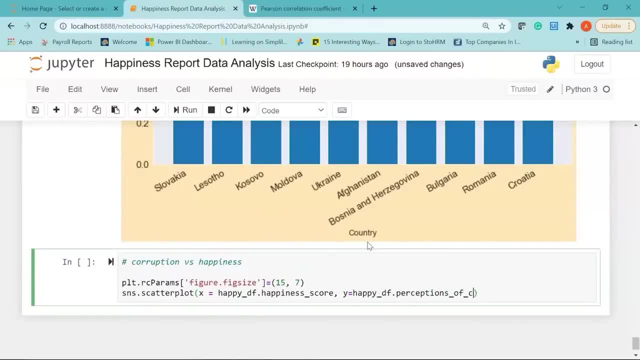 perceptions of corruption. and then in hue we will have the region, that is regional underscore indicator. so i will say happy, underscore, df, dot, regional indicator. and i am going to give the size of the dots. so i will say s equal to 200. then i am going to say: 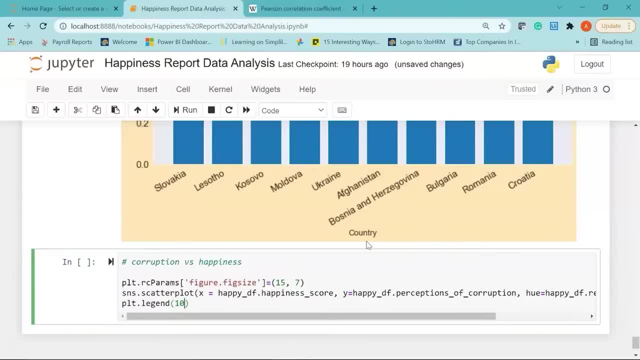 plt dot legend. i am going to put it at lower left corner this time, so i am giving my location as lower left and the font size of the legend i want is 14. after that i will just say plt dot x label as corruption and plt dot. 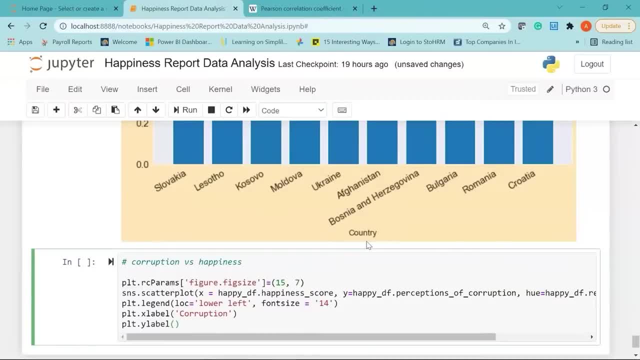 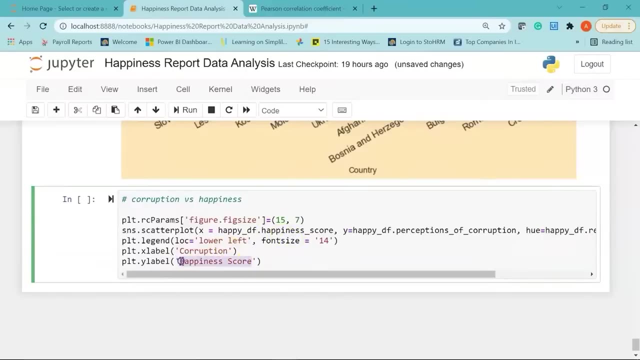 y label and as happiness score. this should rather be the opposite, since in the x axis we have taken happiness score. so we will put the happiness score label in x and i will have corruption in y. alright, so i have my scatter plot code ready, let me just run it. 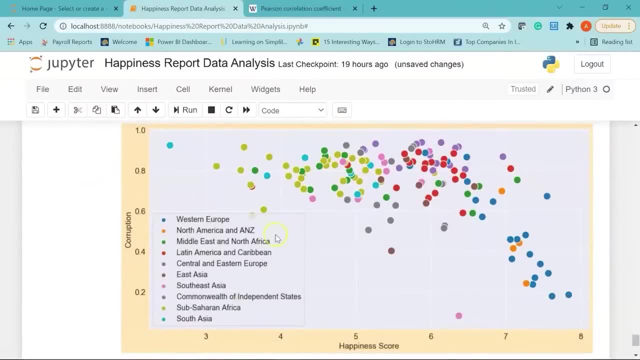 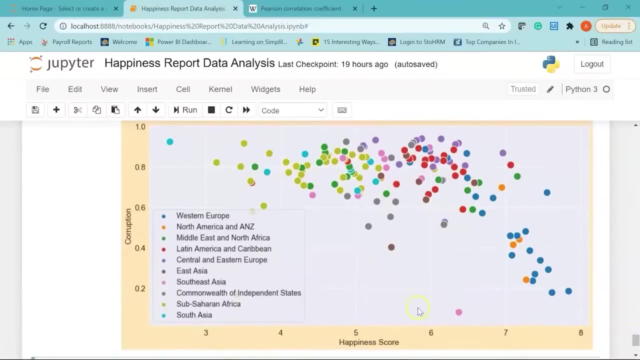 there you go. so here you can see: on the lower left i have the different regions, and on the x axis i have the happiness score. on the y axis i have the corruption index. now you can see the general trend, as per the scatter plot that the countries 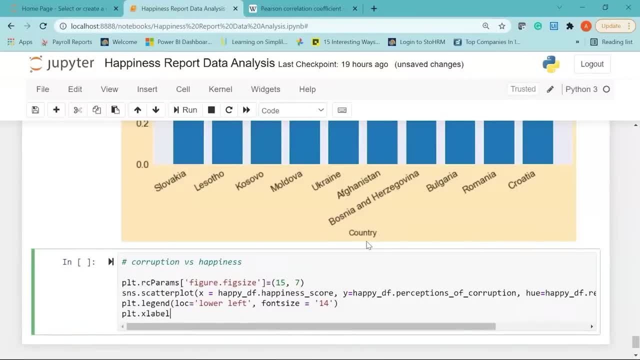 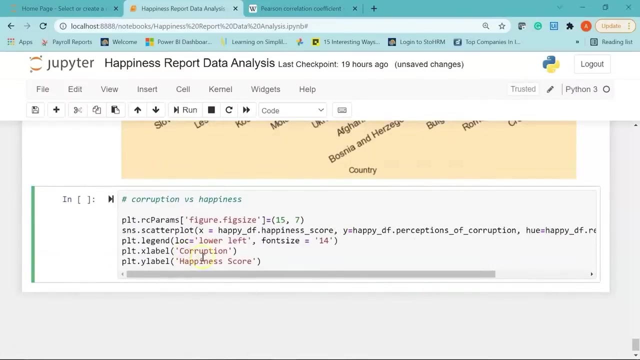 say plt dot x label as corruption and plt dot y label as happiness score. so this should rather be the opposite, since in the x axis we have taken happiness score, so we will put the happiness score label in x and i will have corruption in y. alright, so i have my scatter plot. 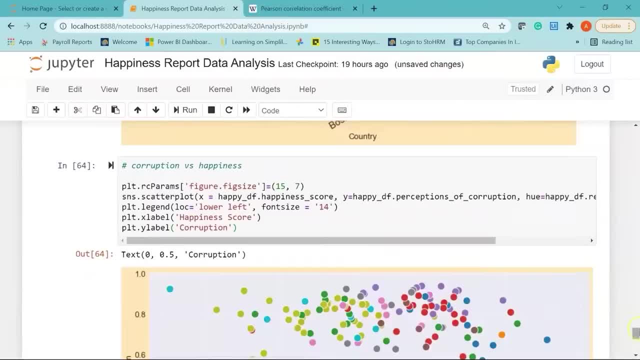 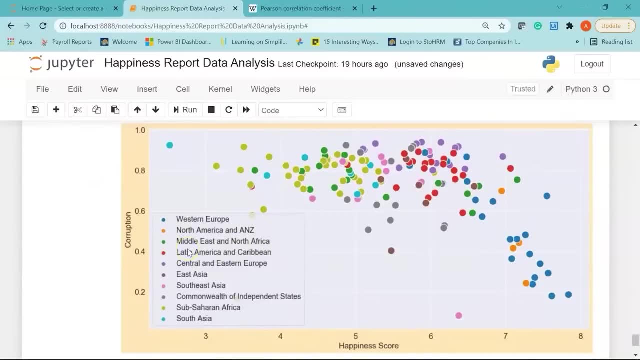 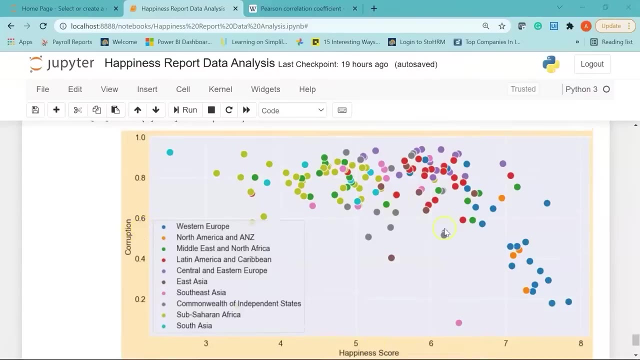 code ready, let me just run it. there you go. so here you can see: on the lower left i have the different regions and on the x axis i have the happiness score. on the y axis i have the corruption index. you can see the general trend as per the scatter. 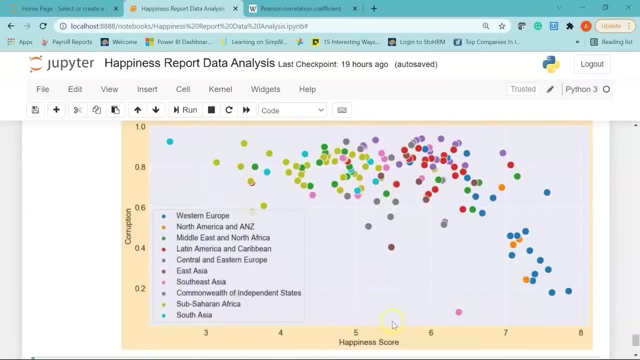 plot that the countries with greater happiness score have lower corruption index. so you can see, these countries which are from the western european regions have highest happiness score and their corruption is also really low. so all these blue countries- you can name a few: finland, we have sweden, we have belgium. 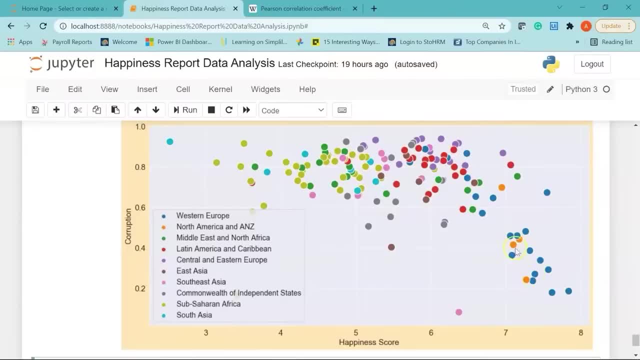 france, netherland, lying in these regions. we also have a few countries from north america and anz, which are essentially australia. then we also have canada, us and new zealand. ok, now, if you focus on these green region, this region, now, these are the countries from the sub. 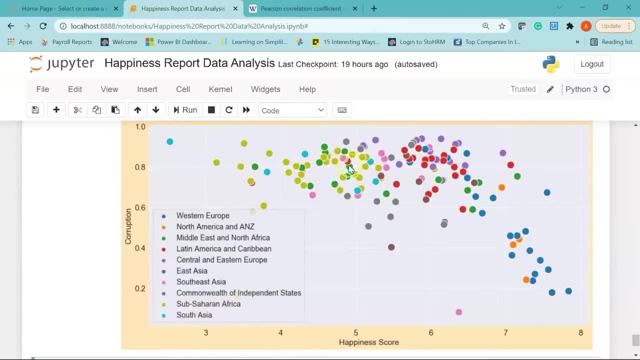 saharan africa and most of the countries from these regions have a very low or less than 5 happiness score. but the corruption is also really high. you can see here they have almost more than 0.7 the corruption index. now you also have a country here which is from the 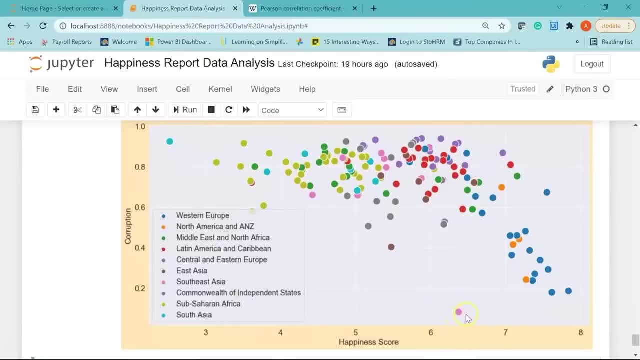 southeast asia. we would like to give you a task. it would be really great if you can tell us in the comment section which country is this. it has more than 6 happiness score, but the corruption index is really low, which is less than 0.2. 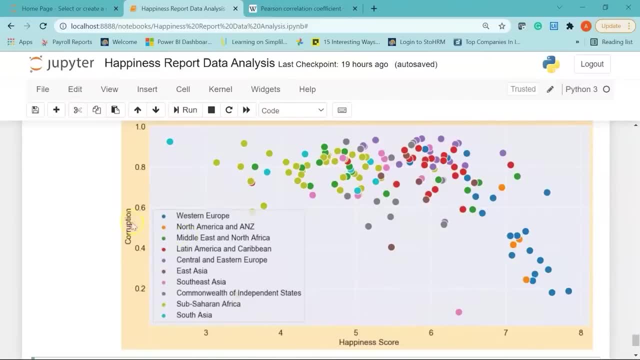 with greater happiness score have lower corruption index. so you can see, these countries which are from the western european regions have highest happiness score and their corruption is also really low. so all these blue countries, you can name a few: finland, we have sweden, we have belgium. 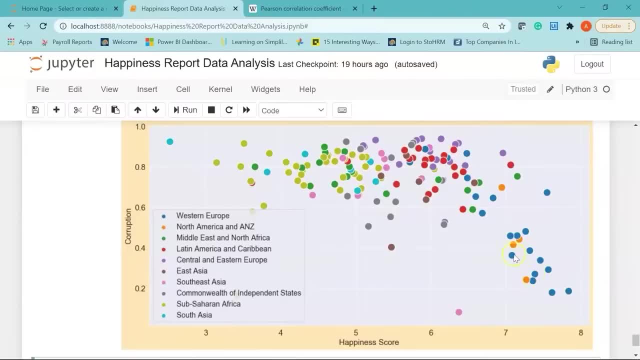 france, netherland, lying in these regions. we also have a few countries from north america and enz, which are essentially australia. then we also have canada, us and new zealand. ok, now, if you focus on these green region, this region, now, these are the countries from the sub. 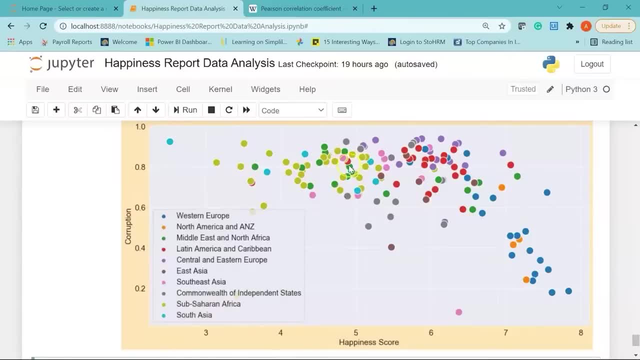 saharan africa and most of the countries from these regions have a very low or less than 5 happiness score. but the corruption is also really high. you can see here they have almost more than 0.7 the corruption index. now you also have a country here which is from the 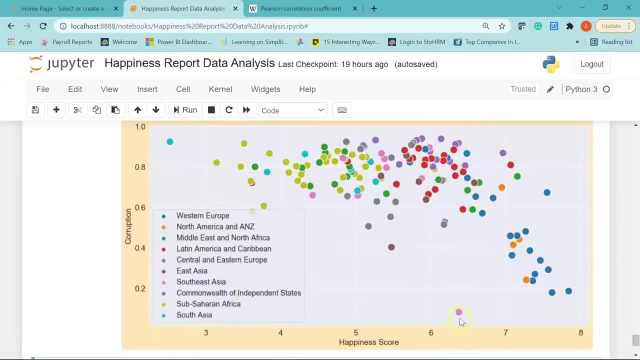 southeast asia. we would like to give you a task. it would be really great if you can tell us in the comment section which country is this. it has more than 6 happiness score, but the corruption index is really low, which is less than 0.2. 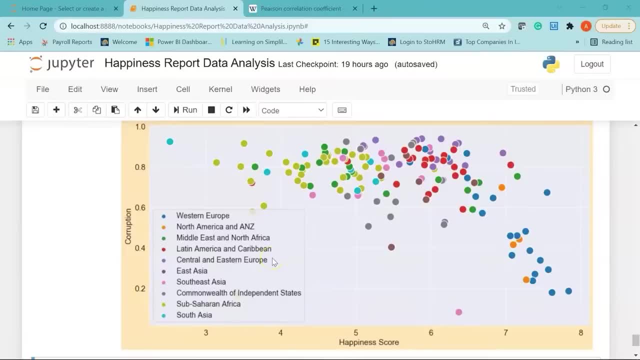 now, if you consider middle east and north african regions, the darker green countries here also, if you see, the happiness score is less than 5 and the corruption index is also high. now there are a few countries, the commonwealth of independent states, for example, countries such as: 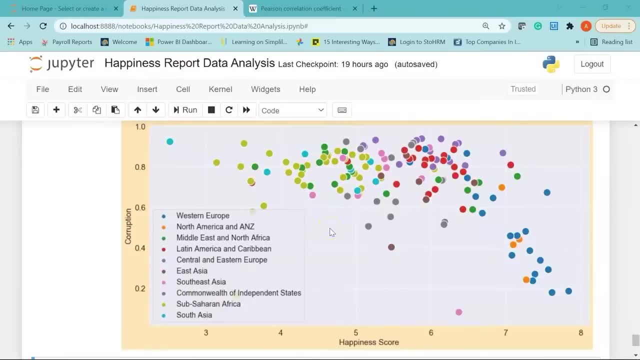 uzbekistan. then you also have kajikistan. we have russia, armenia, belonging to these grey color dots. you also have georgia and ukraine as part of commonwealth of independent states. so here you see, the corruption is below 0.6 for these countries. 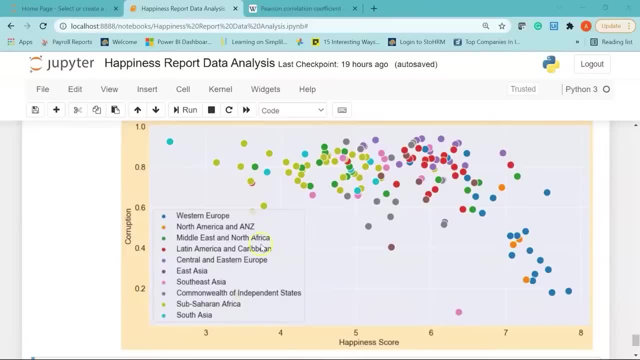 now, if you consider middle east and north africa regions, the darker green countries here also, if you see, the happiness score is less than 5 and the corruption index is also high. now there are a few countries, the commonwealth of independent states, for example, countries such as: 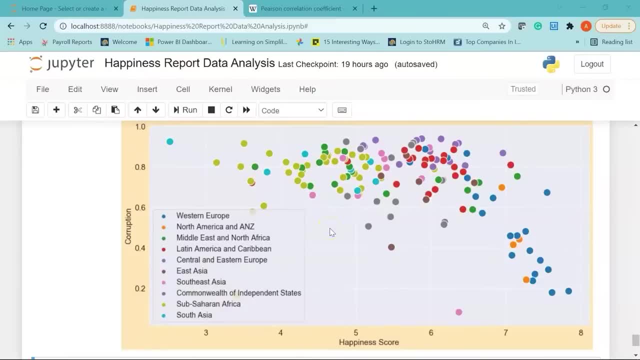 uzbekistan. then you also have kajikistan, we have russia, armenia- belonging to these grey color dots. you also have georgia and ukraine as part of commonwealth of independent states. so here you see, the corruption is below 0.6. 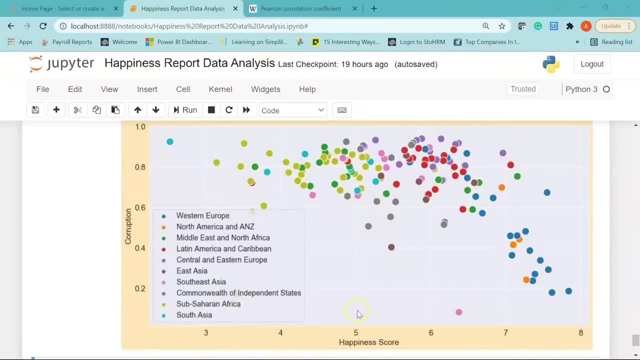 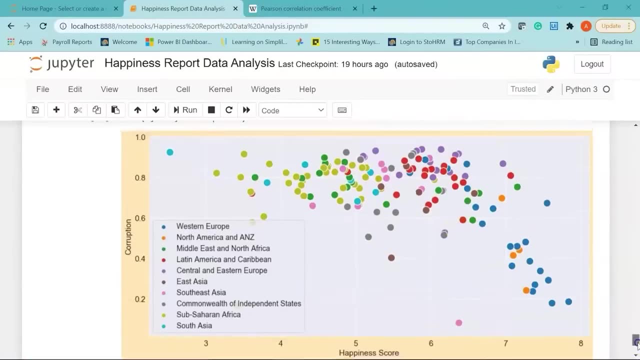 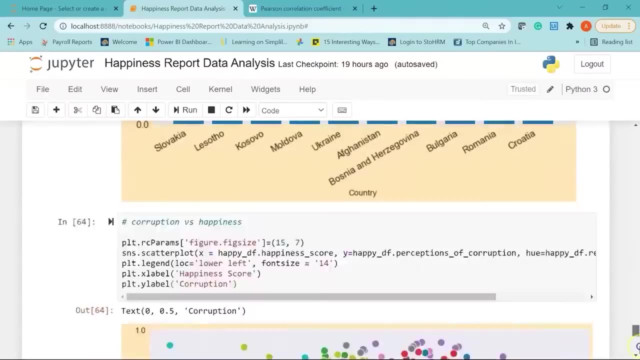 for these countries and the happiness score is more than 5. alright. so with that, we have come to the end of this demo session on world happiness report 2021: data analysis using python. hello everyone, welcome to this exciting video on olympics dataset analysis using python, by simply. 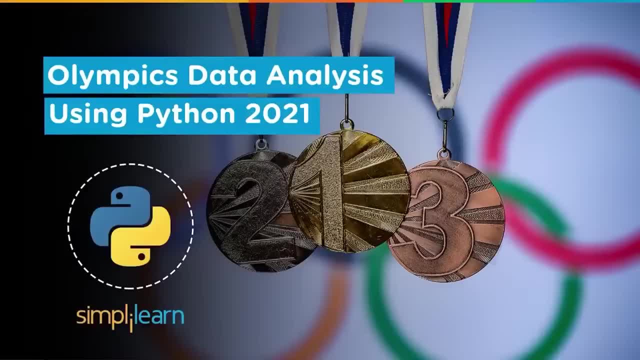 learn. this is going to be a very interesting and interactive session where i will give you a brief about the history of olympics and throw some light into the recently held tokyo olympics, but we will focus more on using olympics dataset that is available on: 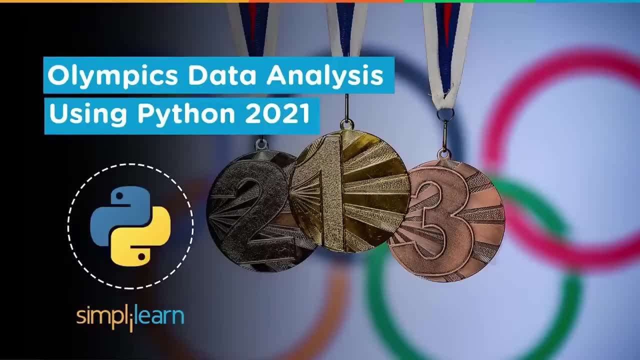 kegel and perform some exploratory data analysis, you will understand how to use different functions in python to analyze and extract meaningful information. during the course of our discussion, i will be asking you a few general questions related to the olympics. try to answer them in the 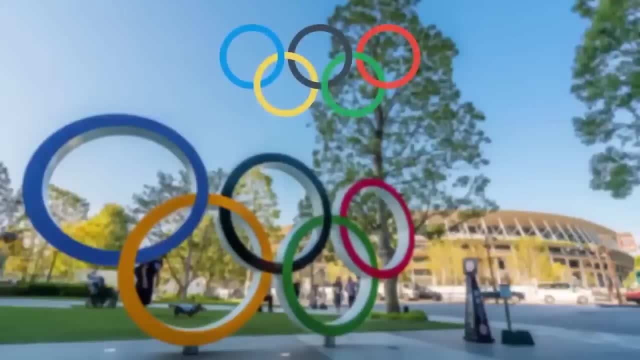 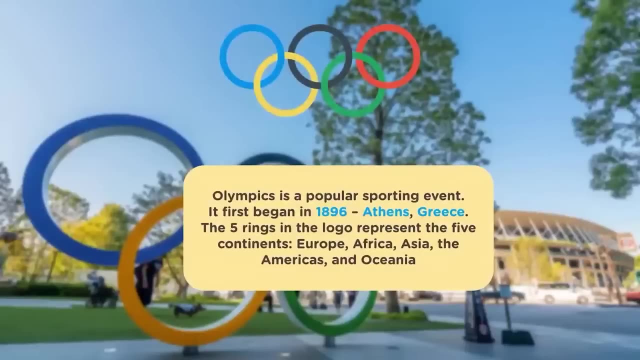 comment section of the video. so let's begin. the olympics is one of the biggest sporting events on the planet. it is held every four years. the first modern olympics took place in athens, greece, in 1896. as per national geographic, the original. 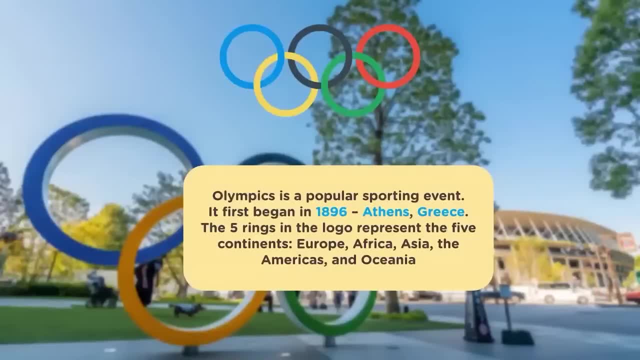 olympics took place in 776 bc, so they began as part of an ancient greek festival which celebrated the greek god of sky and weather. the rings in the olympics logo represent the five continents: europe, africa, asia, the americas and oceania. 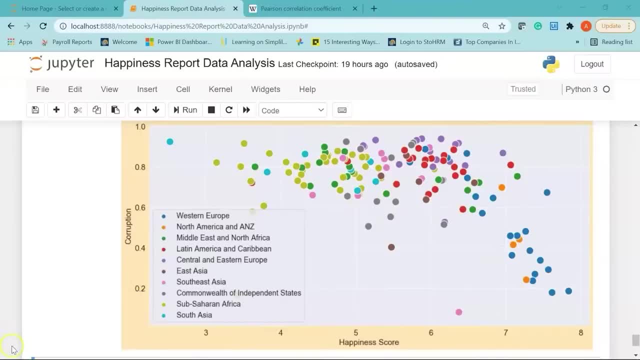 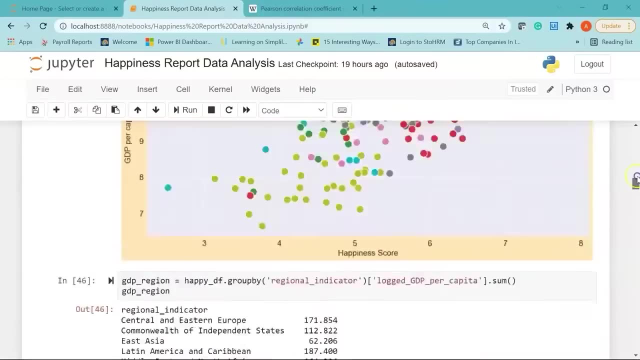 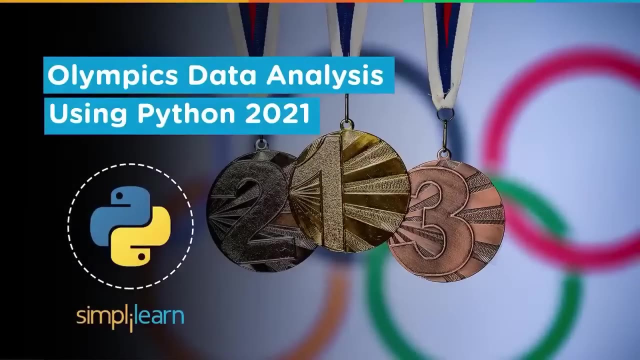 and the happiness score is more than 5. alright, so with that, we have come to the end of this demo session on world happiness report 2021. data analysis using python. hello everyone, welcome to this exciting video on olympics dataset analysis using python by simply learn. 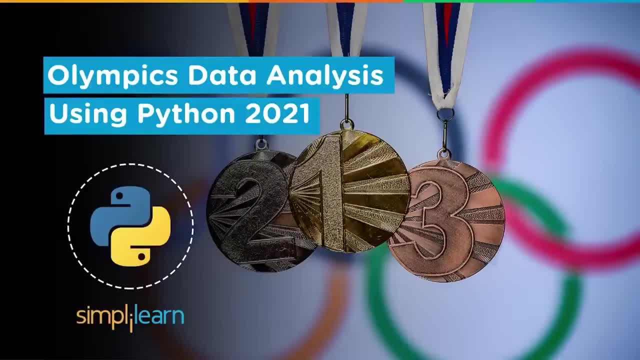 this is going to be a very interesting and interactive session where i'll give you a brief about the history of olympics and throw some light into the recently held tokyo olympics, but we'll focus more on using olympics dataset that is available. 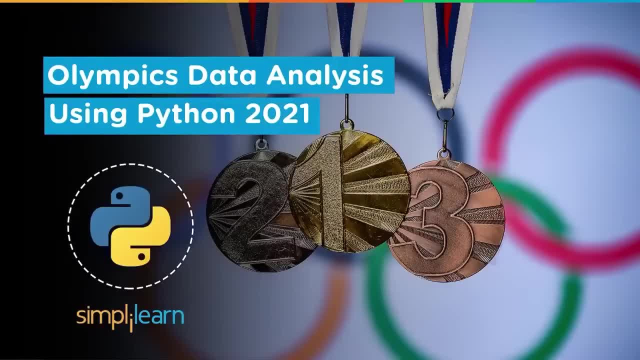 on kegel and perform some exploratory data analysis, you will understand how to use different functions in python to analyze and extract meaningful information. during the course of our discussion, i'll be asking you a few general questions related to the olympics. try to answer them in the 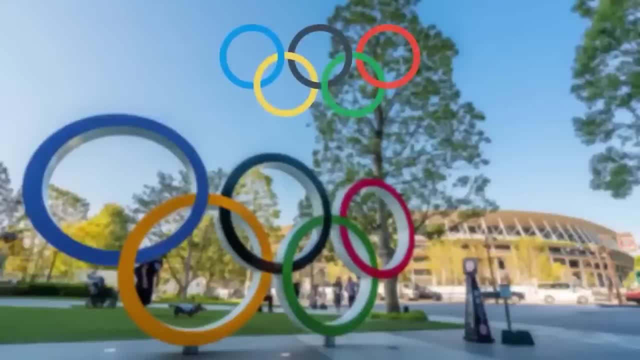 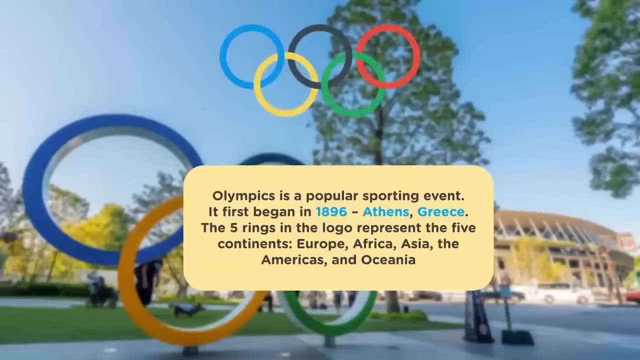 comment section of the video. so let's begin. the olympics is one of the biggest sporting events on the planet. it is held every four years. the first modern olympics took place in athens, greece, in 1896. as per national geographic, the 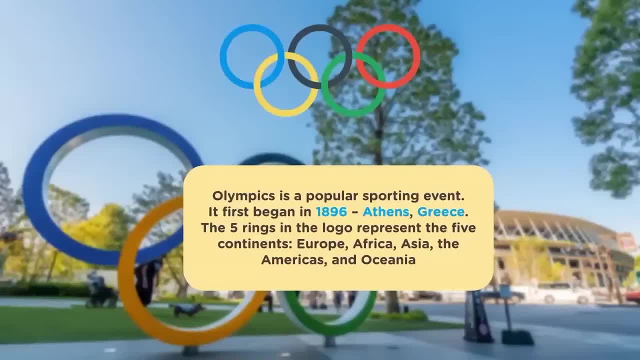 original olympics took place in 776 bc, so they began as part of an ancient greek festival which celebrated jews, the greek god of sky and weather. the rings in the olympics logo represent the five continents: europe, africa, asia, the americas and. 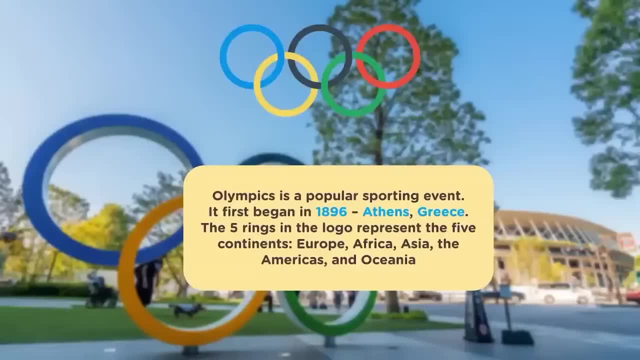 oceania from 1924 to 1992. the winter and the summer. olympics took place in the same year, but now they alternate every two years. before i move on, here is an interesting question for you. only two people have ever won gold medals. 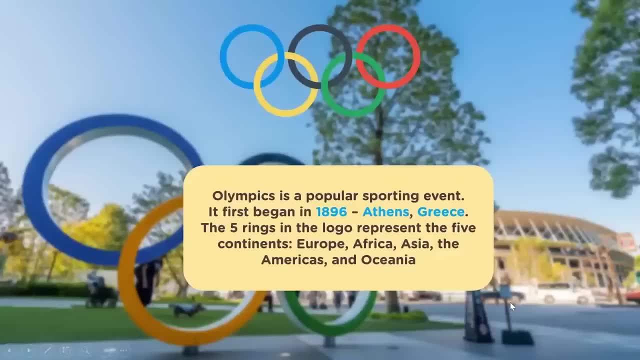 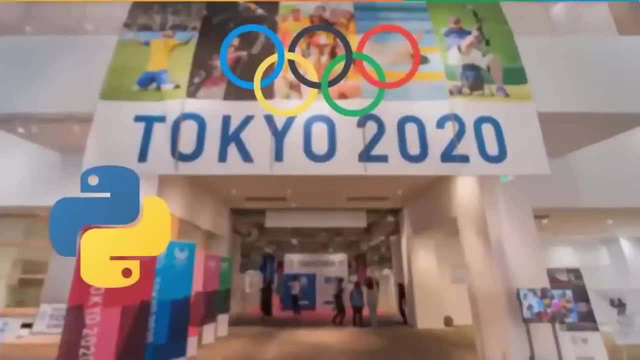 at both the summer and the winter olympics. who are those two people? please share your answers in the comment section of the video. we would like to know from you. the summer olympics in tokyo began on the 23rd of july and recently concluded, on the 8th. 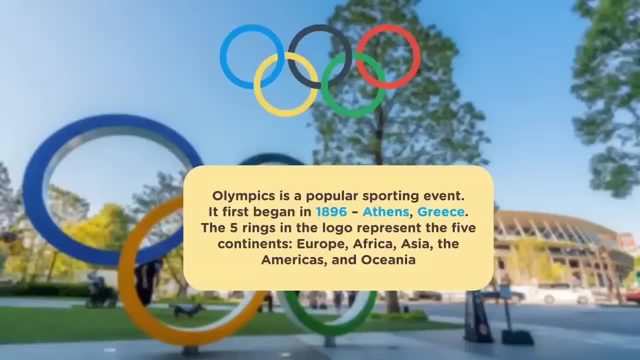 from 1924 to 1992, the winter and the summer olympics took place in the same year, but now they alternate every two years. before i move on, here is an interesting question for you. only two people have ever won gold medals at both the summer and the winter olympics. 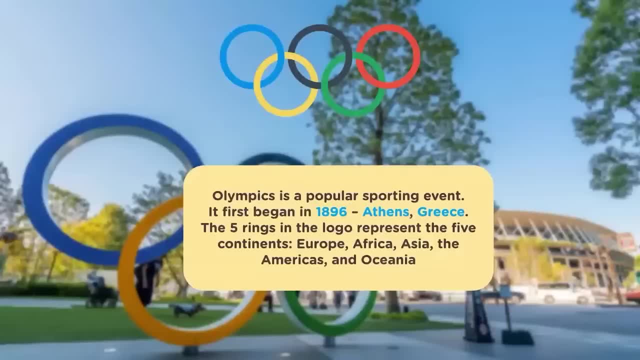 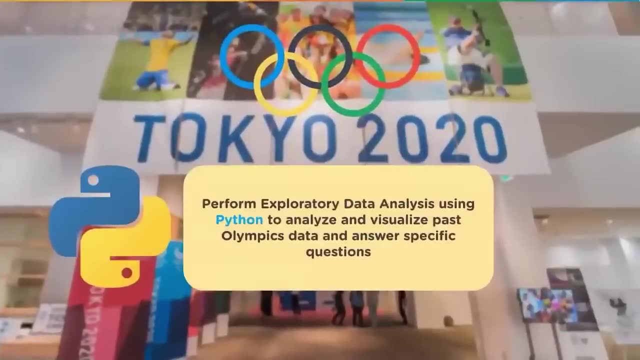 who are those two people? please share your answers in the comment section of the video. we would like to know from you. the summer olympics in tokyo began on the 23rd of july and recently concluded, on the 8th of august. 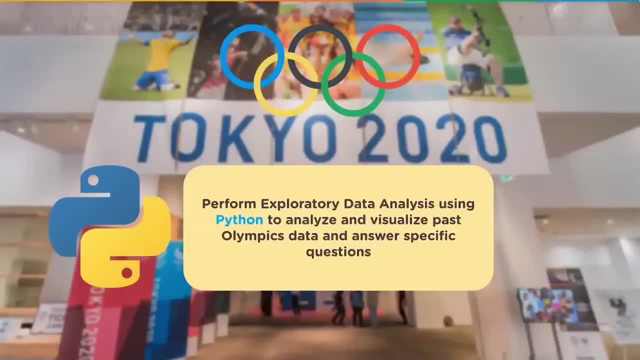 we got to witness some thriller matches that went down to the wire, some amazing victories and, sadly, there were a lot of heartbreaks as well. winning and losing are part and parcel of any game. fans across the world were really happy to see this global event happen this year, following last years. 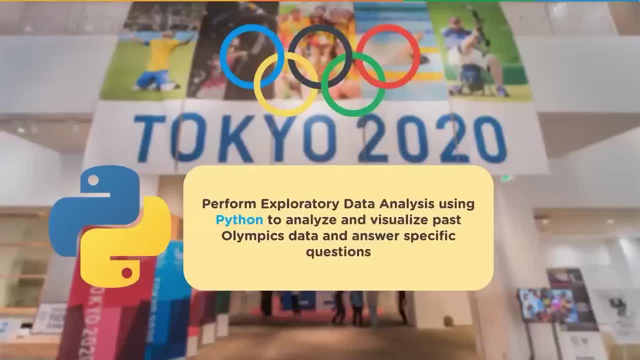 tournament due to the coronavirus pandemic. with our olympic fever high, lets take this opportunity to work around a project to perform exploratory data analysis using python to analyze and visualize past olympics data and answer specific questions. in this video, we will be using specific python. 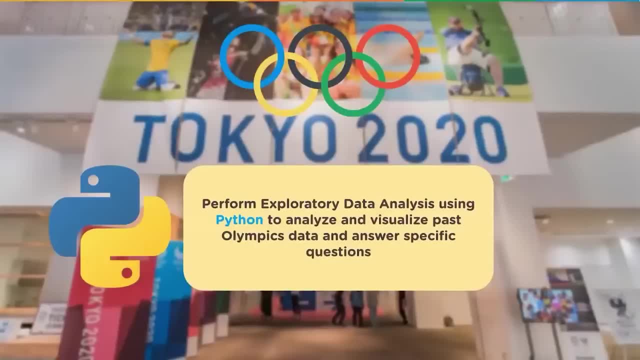 libraries such as numpy, pandas, matplotlib and seaborn to make sense of our data and extract meaningful information. we are going to visualize our results with different charts and graphs. before i show you the data set that we are going to use for our analysis, i have another general question for you. which is the first olympics where all the participating countries sent female athletes. i repeat, which is the first olympics where all the participating countries sent female athletes. put the year and the city name where the olympics was held in the comment section of the video. 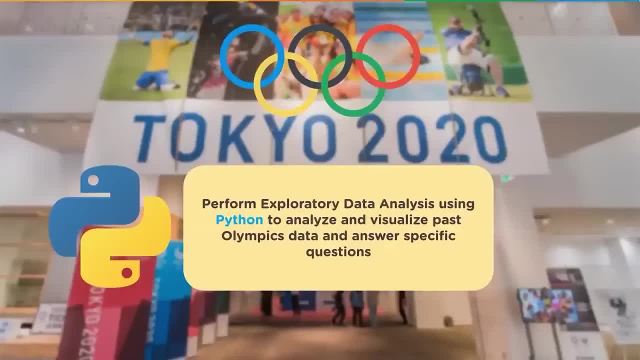 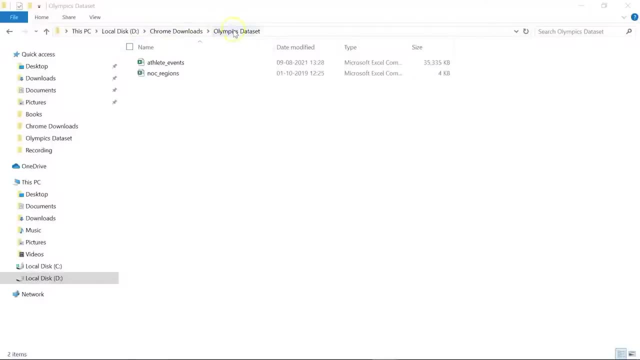 we will be more than happy to hear from you. now let me go ahead and show you the data sets that we will be using in this video. so here you can see. i have my olympics data set folder that has two data sets. these are csv files. one is called the 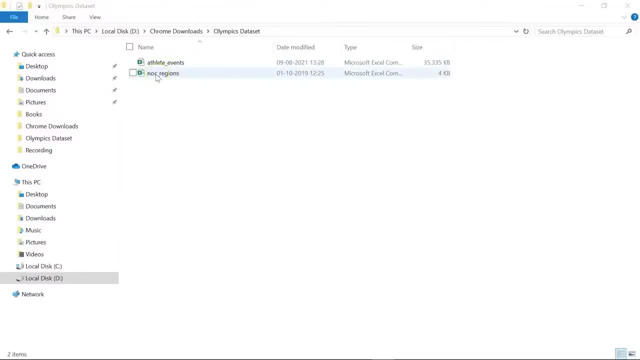 athlete underscore events and the other one is called noc underscore regions. so we will be using these two data sets. these data sets can be downloaded from kegel. we will post the data set links in the description of the video. please go ahead and download them. these data sets have been directly. 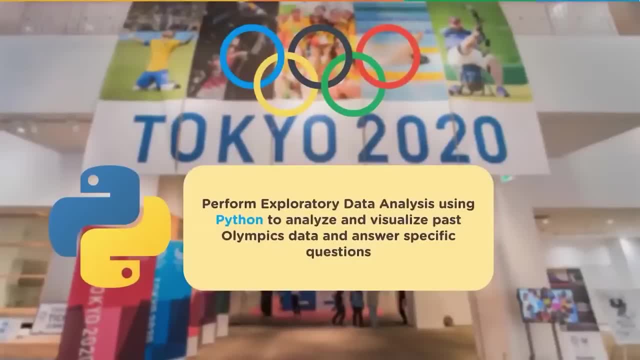 of august, we got to witness some thriller matches that went down to the wire, some amazing victories and, sadly, there were a lot of heartbreaks as well. winning and losing are part and parcel of any game. fans across the world were really happy to see this global. 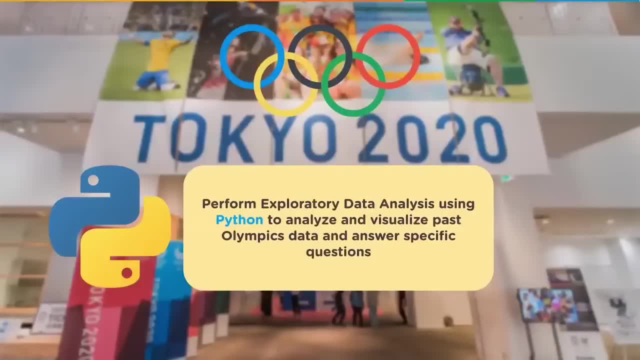 event happen this year, following last year's postponement due to the coronavirus pandemic. with our olympic fever high, let's take this opportunity to work around a project to perform exploratory data analysis using python to analyze and visualize past olympics data and answer. 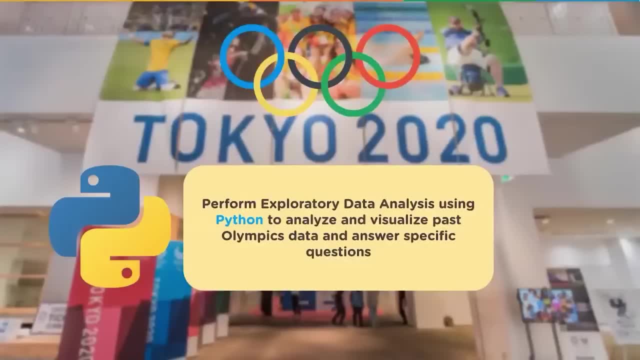 specific questions in this video. we will be using specific python libraries, such as numpy, pandas, matplotlib and seaborn, to make sense of our data and extract meaningful information. we are going to visualize our results with different charts and graphs before i show you the data set that we are going to use for our analysis. i have another general question for you, which is the first olympics where all the participating countries sent female athletes. i repeat, which is the first olympics where all the participating countries sent female athletes. put the year and the city name where the olympics was. 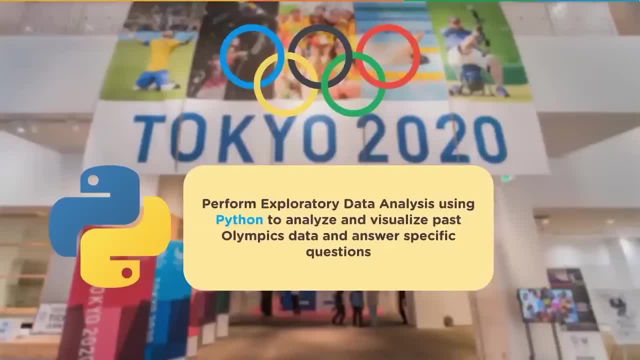 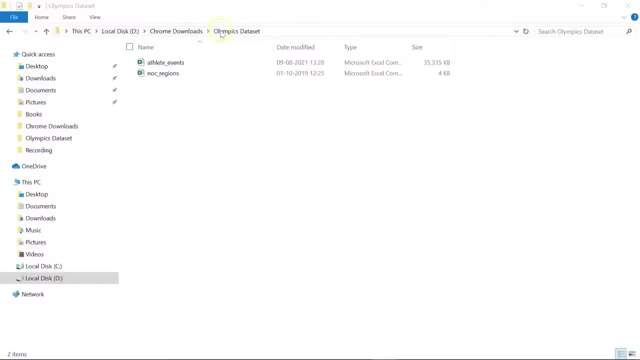 held in the comment section of the video. we'll be more than happy to hear from you. now let me go ahead and show you the data sets that we'll be using in this video. so here you can see i have my olympics data set folder that. 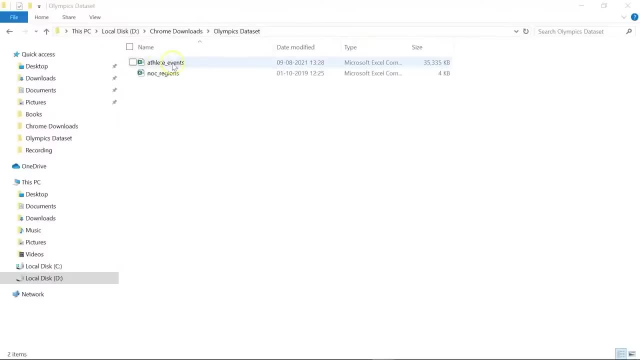 has two data sets. these are csv files. one is called the athlete underscore events and the other one is called noc underscore regions. so we'll be using these two data sets. these data sets can be downloaded from kegel. we will post the data set links in the description of the. 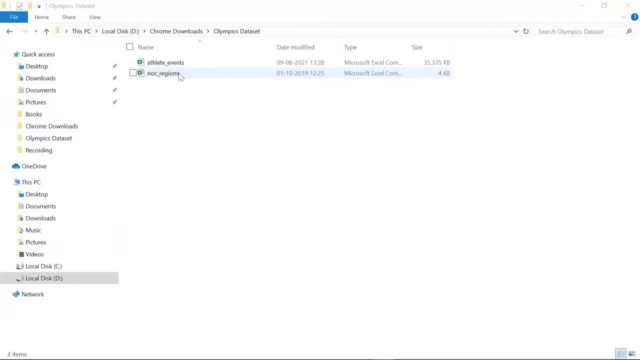 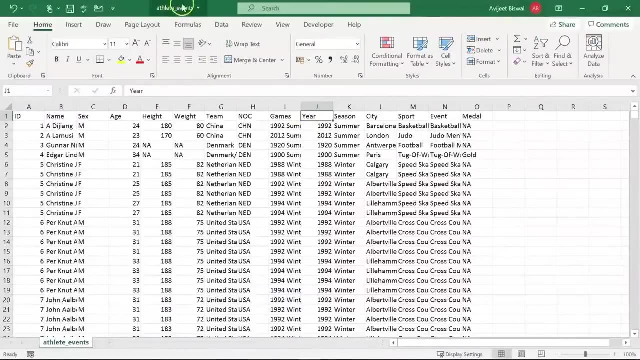 video. please go ahead and download them. these data sets have been directly taken from the internet. now i'll show you the data sets. so this is my first data set. you can see on the top athlete underscore events. so i have around 15 columns. you can see the count here. 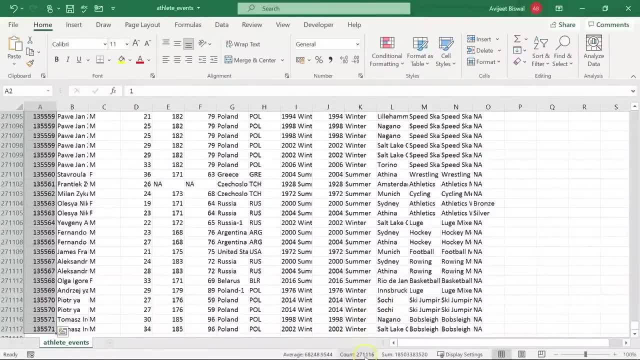 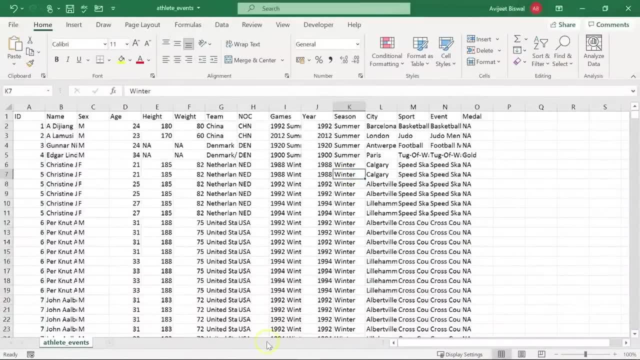 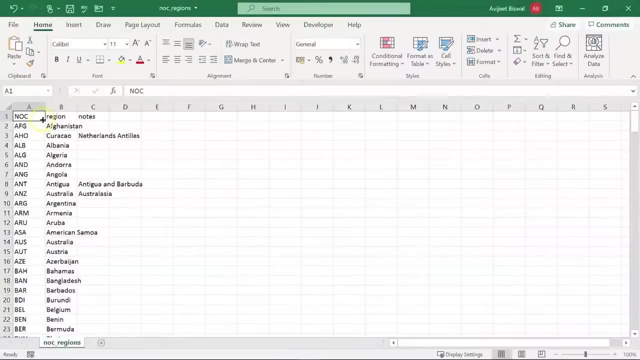 and there are nearly 271116 rows of information. so this is a huge data set that we are going to use. the other data set we are going to use in this demo is called noc underscore regions. now here, one thing to notice: noc stands for national olympic committee. 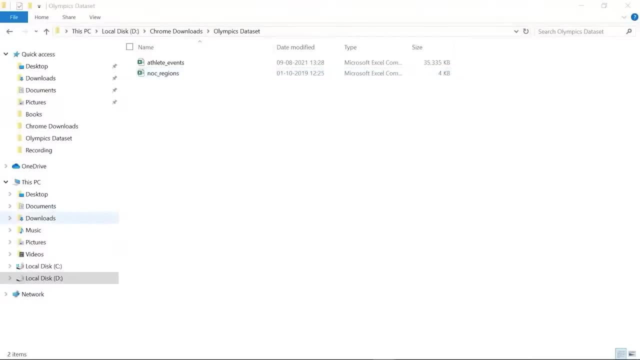 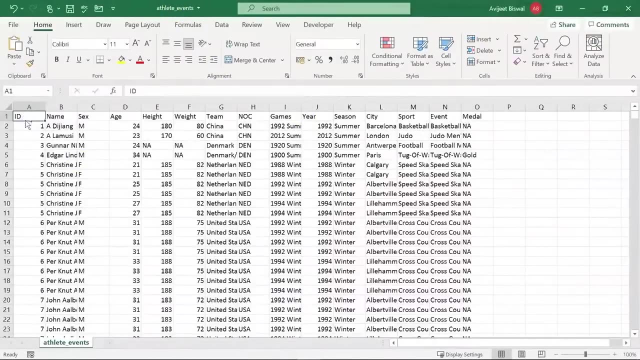 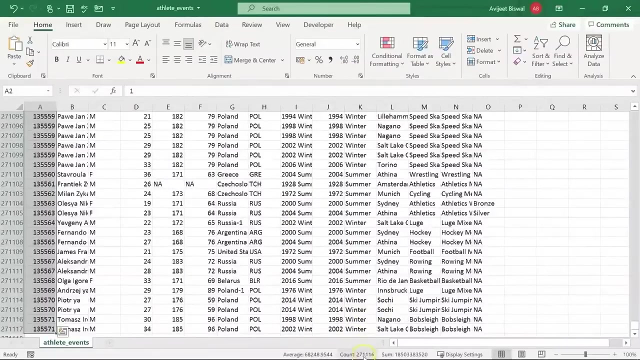 taken from the internet. now i will show you the data sets. so this is my first data set. you can see on the top athlete underscore events. so i have around 15 columns- you can see the count here- and there are nearly two lakh seventy one thousand one hundred and sixteen rows. 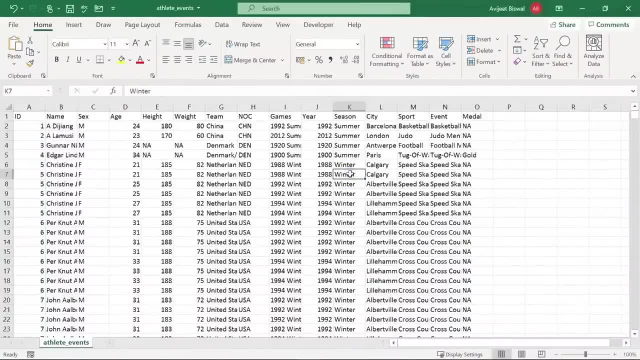 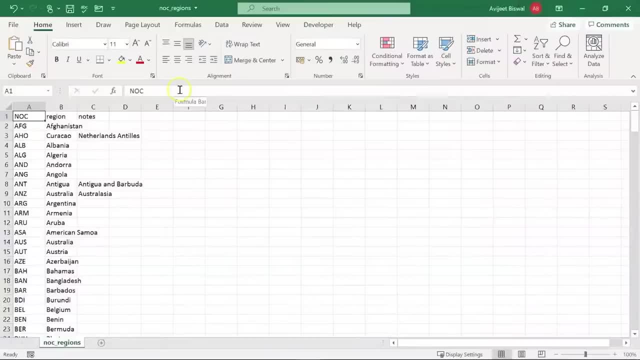 of information. so this is a huge data set that we are going to use. the other data set we are going to use in this demo is called noc- underscore regions. now here, one thing to notice: noc stands for national olympic committee. this is a three letter code that is given by 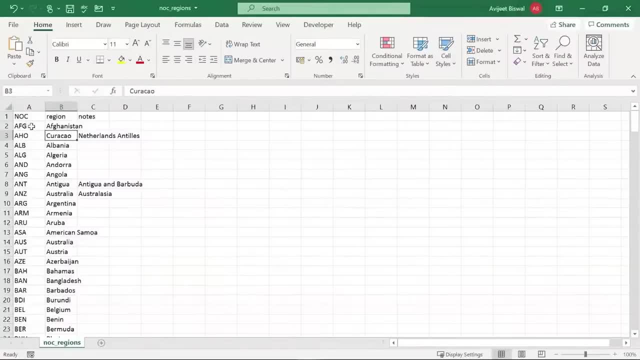 the olympic committee. we have the region names. so afg is for afghanistan, you have alb for albania, alg for algeria. we have also a column called notes. you find some notes about the region. for example here, antiqua is actually. 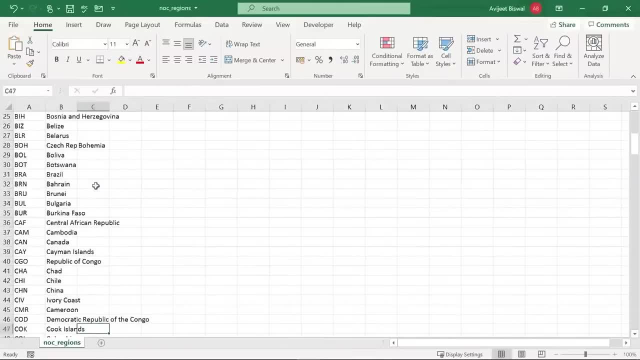 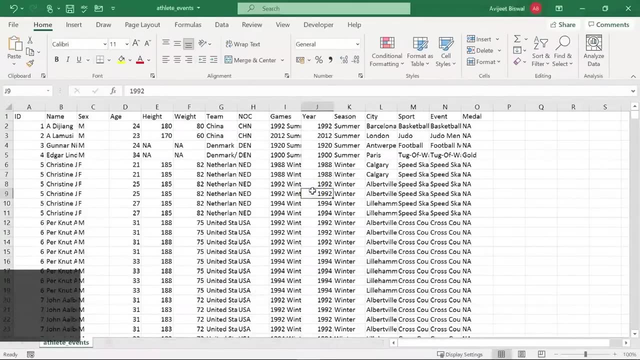 antiqua and barbuda. alright, let's move to the first data set that i showed you. this is a primary data set for our demo, so these data sets have been directly taken from the internet and were not validated, so the results that you will see in the demo is purely based on. 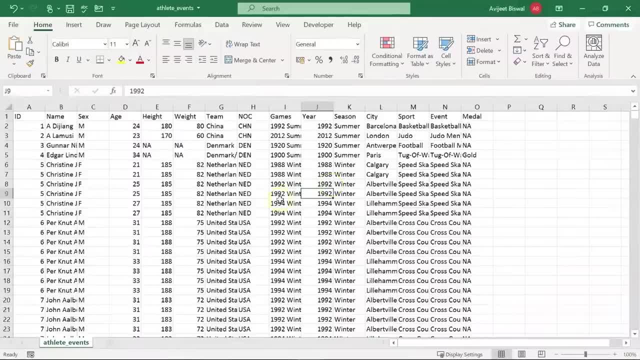 the data that we have collected. so the file athlete underscore events dot csv contains nearly two lakh seventy one thousand one hundred and sixteen rows of information, and there are fifteen columns. so each row corresponds to an individual athlete competing in an individual olympic event. so here, 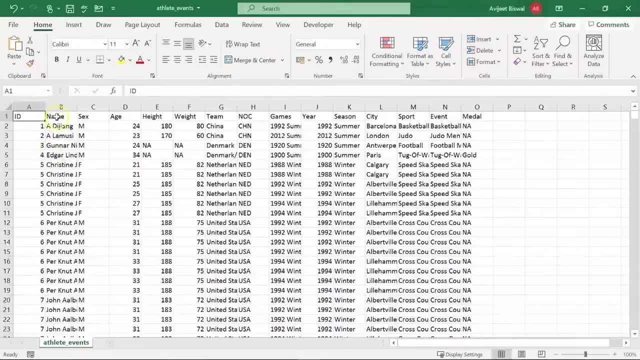 id is actually a unique number for each athlete. then we have the name, which is basically the athlete's name. we have the sex or the gender, which is male or f for female. then we have the age of the athlete, which is in terms of integers. we have the 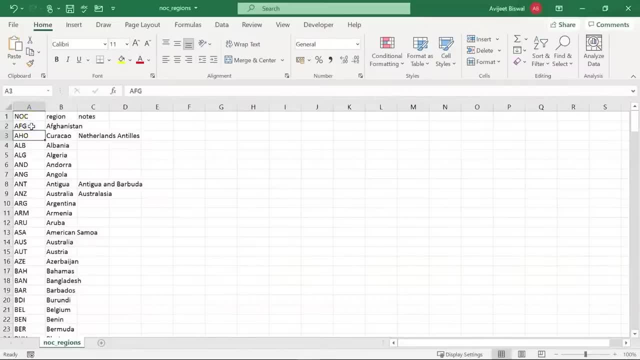 this is a three letter code that is given by the olympic committee. we have the region names, so afg is for afghanistan. you have alb for albania, alg for algeria. we have also a column called notes. you find some notes. 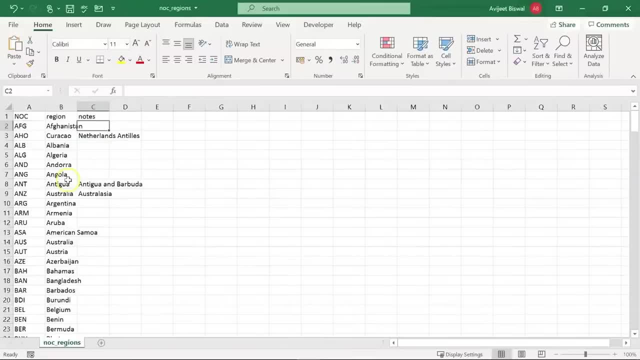 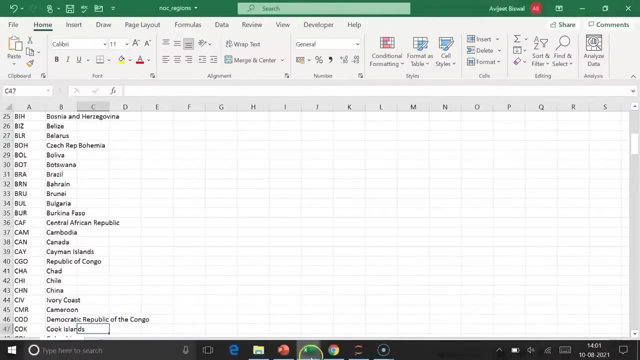 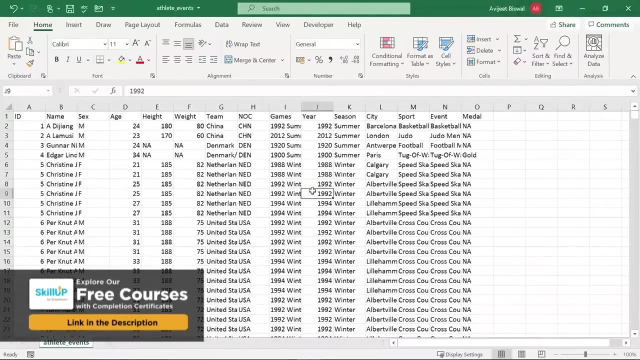 about the region. for example, here antiqua is actually antiqua and barbuda. all right, let's move to the first data set that i showed you. this is our primary data set for our demo, so these data sets have been directly taken from the internet, and. 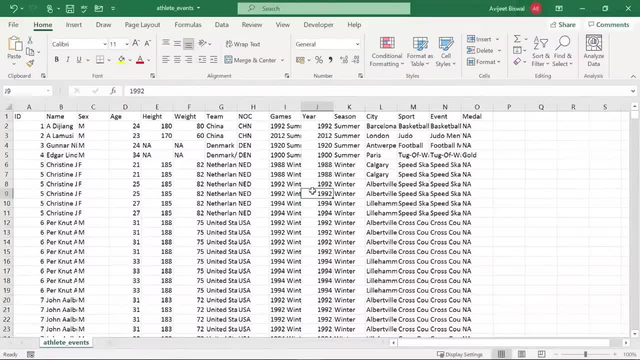 were not validated, so the results that you will see in the demo is purely based on the data that we have collected. so the file athlete underscore events dot csv contains nearly 271116 rows of information and there are 15 columns, so each row corresponds to an individual. 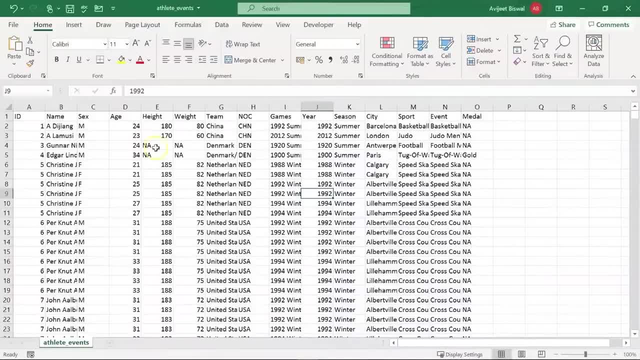 athlete competing in an individual olympic event. so here id is actually a unique number for each athlete. then we have the name, which is basically the athlete name. we have the sex or the gender, which is male or f for female. then we have the age of the athlete, which is in terms of. 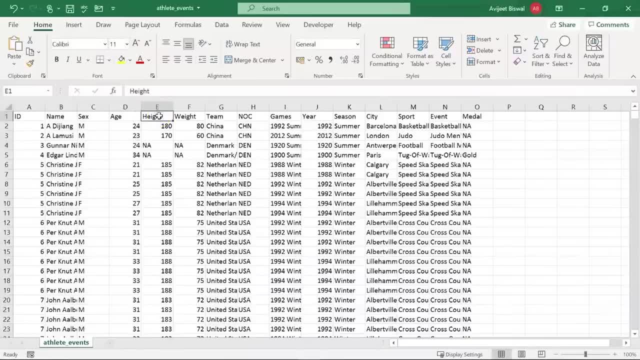 integers. we have the height in centimeters of the athletes, then we have the weight in kilograms. we have the team name. these are the country names. we have china, denmark, netherland. there are around 200 country names. then we have the noc, as i said, noc. 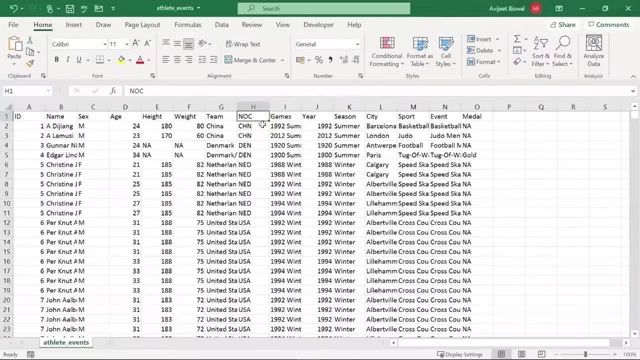 is a three letter code that stands for national olympic committee. we have the games. this games contains the year and the season. you can see here: 1992, summer. you also have the winter olympic information. alright, then we have a specific year column to. 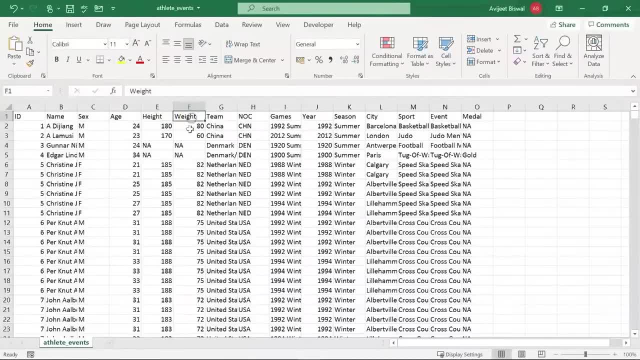 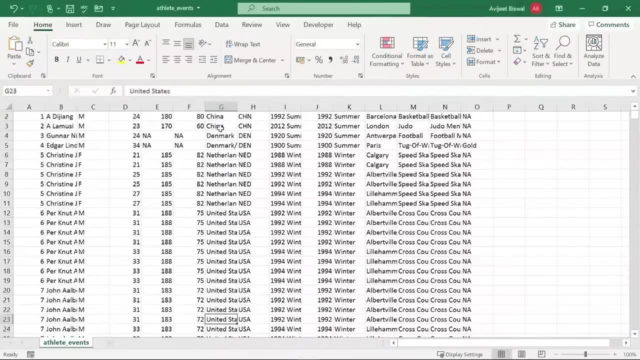 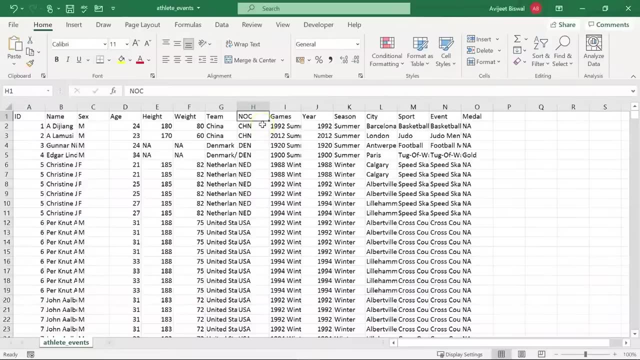 height in centimeters of the athletes. then we have the weight in kilograms. we have the team name. these are the country names. we have china, denmark, netherland. there are around two hundred country names. then we have the noc. as i said, noc is a three letter code that stands for 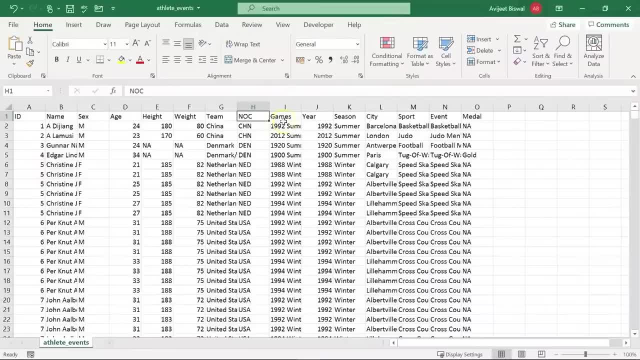 national olympic committee. we have the games. this games contains the year and the season. you can see here nineteen, ninety, two, summer, you also have the winter olympic information, alright, then we have a specific year column to tell you in which year this event had occurred. 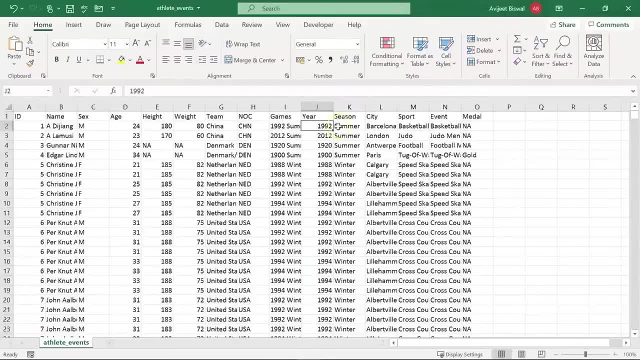 now the year column is also an integer column. we have the season, so whether it was summer olympics or winter olympics. then we have the city name. this is the host city. then we have the sport name. you can see here we have basketball, judo, football, tug of war. 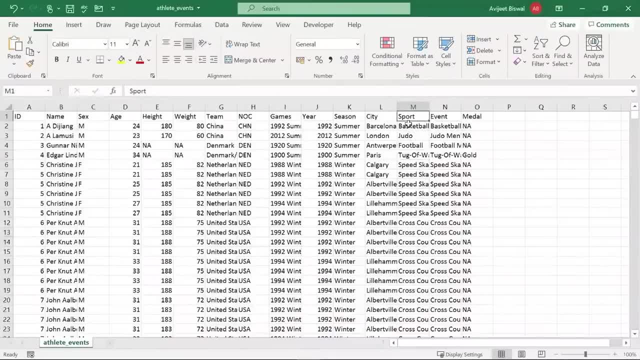 speed skating- there are so many. then we have another column called event, which is the complete event name. as you can see, the sport name is basketball, but the event name is basketball, men's basketball, to be very specific. again, for speed skating you have different categories, like women's. 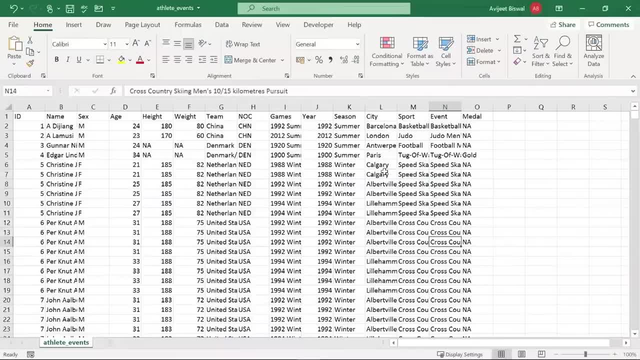 thousand meters, five hundred meters. alright, now the final column is the medal column, so it has the information about the athlete, whether the athlete had won a medal, be it gold, silver, bronze and any means. the athlete did not win any medals, so we will use these two data sets. now let's 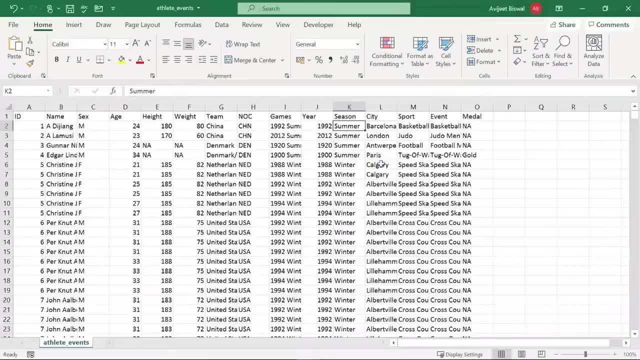 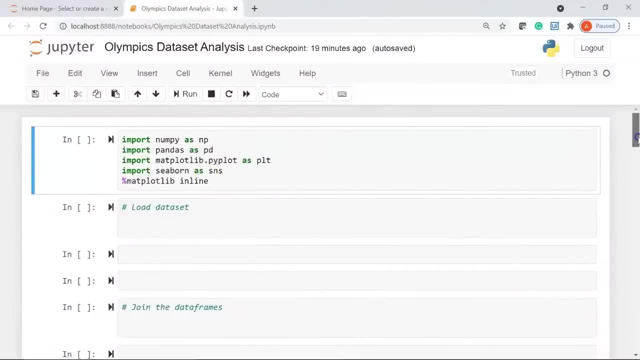 get started with the demo. we will be using jupiter notebook for our analysis, so i will take you to my jupiter notebook right away. i have opened it on chrome, so this is my jupiter notebook that we are going to use. you can see here olympics data. 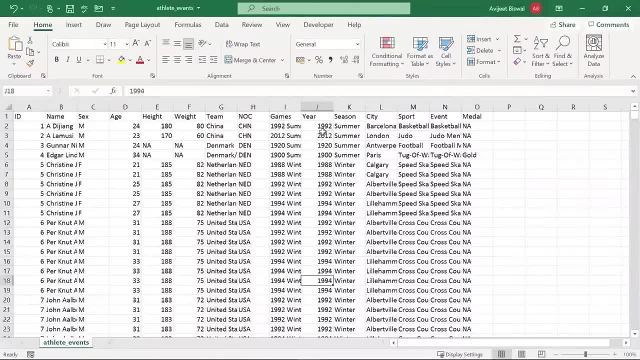 tell you in which year this event had occurred. now, the year column is also an integer column. we have the season, so whether it was summer olympics or winter olympics. then we have the city name: this is the host city. then we have the sport. 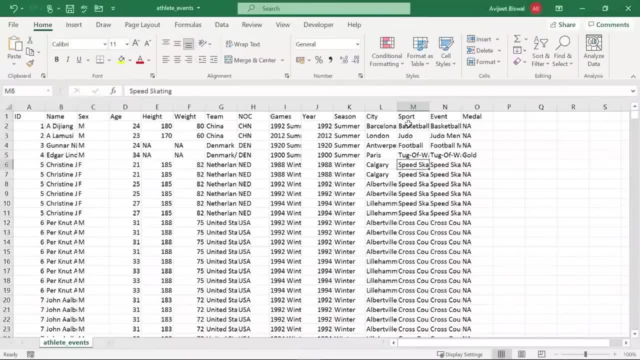 name. you can see here we have basketball, judo football, tug of war, speed skating. there are so many. then we have another column called event, which is the complete event name. as you can see, the sport name is basketball, but the event name is basketball- men's basketball, to be very. 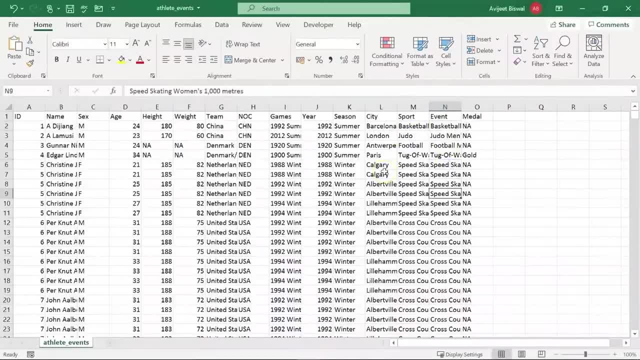 specific again, for speed skating you have different categories, like women's 1000m, 500m. alright, now the final column is the medal column, so it has the information about the athlete, whether the athlete had won a medal, be it gold, silver, bronze and any means. the athlete did not win any. 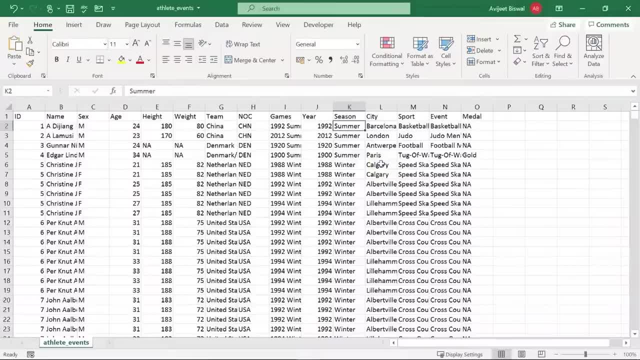 medals. so we will use these two data sets. now let's get started with the demo. we will be using jupiter notebook for our analysis, so i will take you to my jupiter notebook right away. i have opened it on chrome, so this is my jupiter notebook that we are 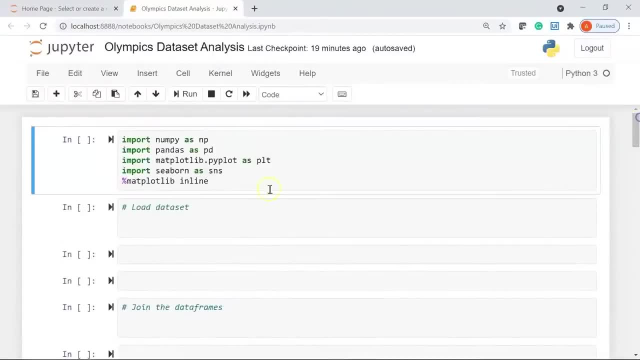 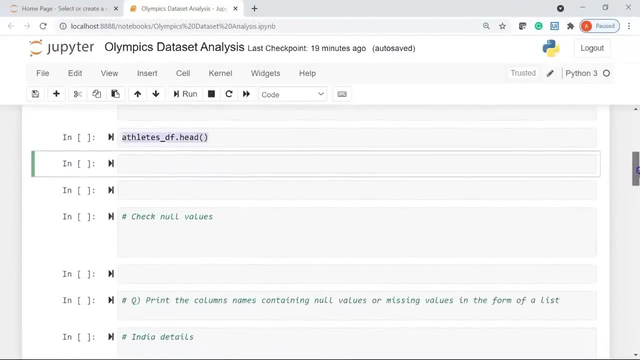 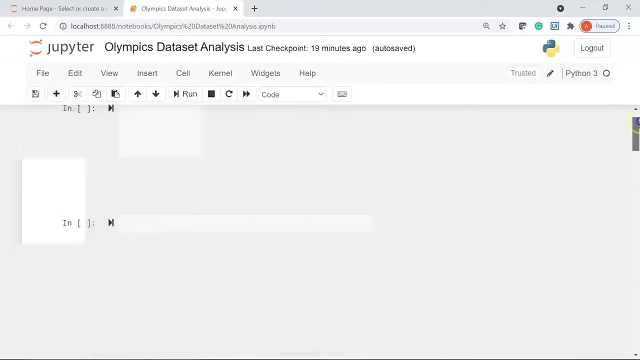 going to use. you can see here olympics dataset analysis. i have already have a few cells that have been filled with some piece of code and you can see there are some comments written as well. we are going to use this dataset, so let's get started. 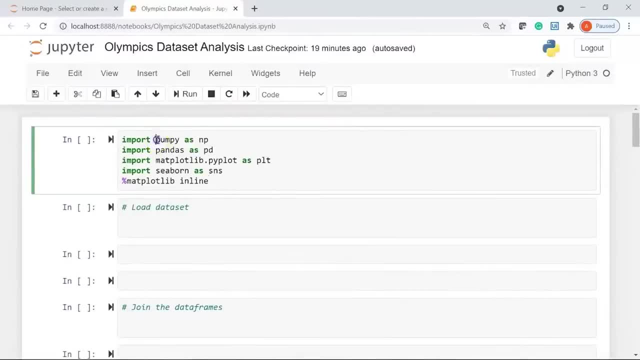 first and foremost, we will import the datasets. so we are going to use numpy, pandas, matplotlib and seaborn. let me hit shift, enter to import all the libraries. alright, now the next thing is to load the datasets using pandas, read, underscore csv function. so i will create a variable called 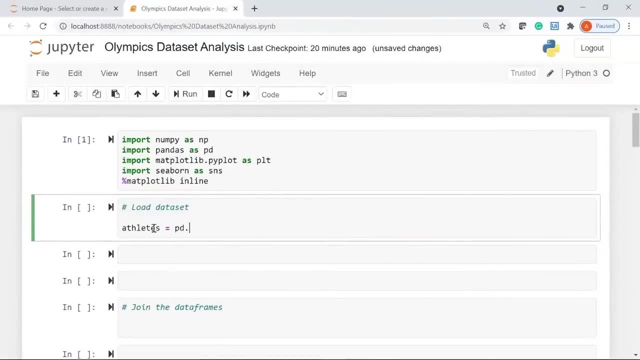 athletes, i will say equal to pd dot. i will use the read underscore csv function and inside this function we will give the location of the files. so i will copy this location and here i will paste. make sure this is within quotations. and these are all forward slash. 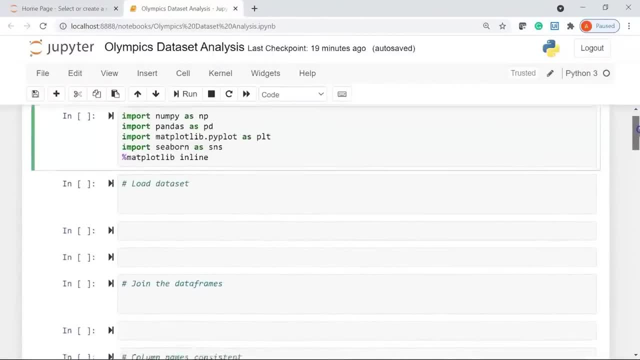 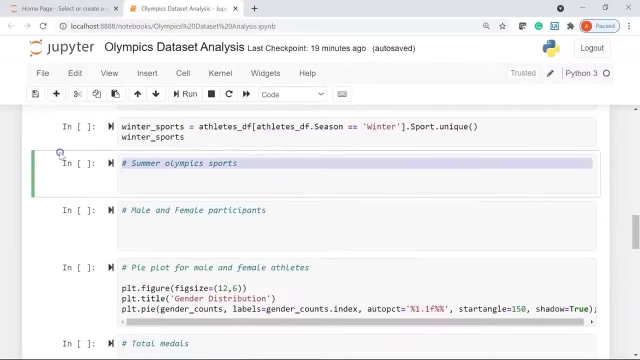 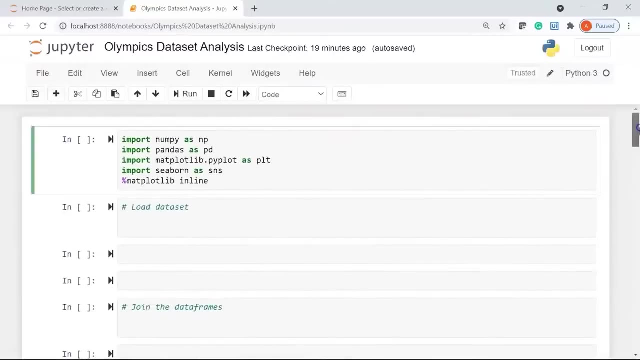 set analysis. i have already have a few cells that have been filled with some piece of code and you can see there are some comments written as well. we are going to use this data set, so let's get started. first and foremost, we will import the data sets, so we are going to use 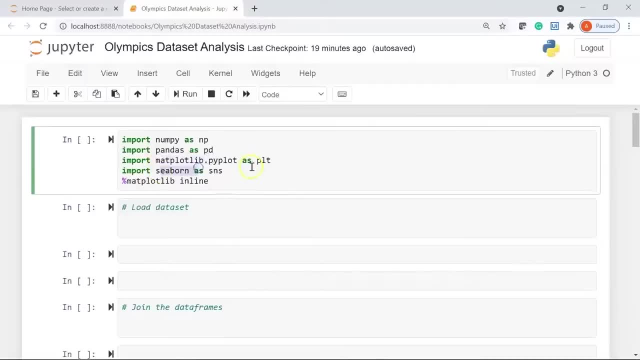 numpy, pandas, matplotlib and seaborn. let me hit shift enter to import all the libraries. alright, now the next thing is to load the data sets using pandas read underscore csv function. so i will create a variable called athlete. i will say equal to pd dot. i will use the read underscore csv. 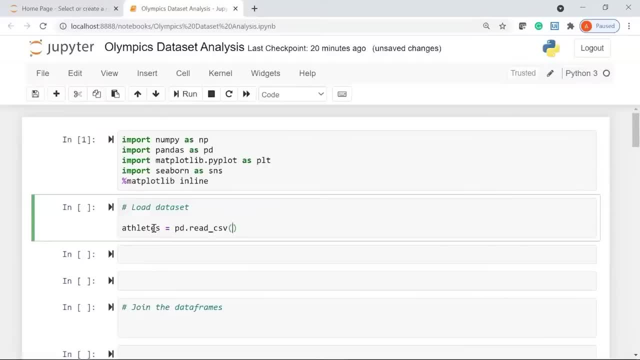 function and inside this function we will give the location of the files. so i will copy this location and here i will paste. make sure this is within quotations and these are all forward slash. give another forward slash and after that i will give the file name, that is. 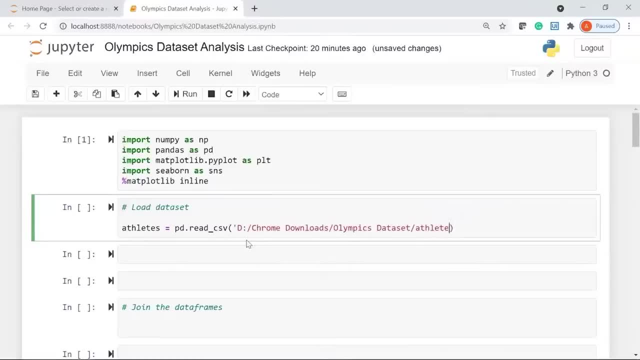 athlete underscore events dot csv. i will close the quotation. let's run it okay. similarly, we will load the second data set. i will create another variable called regions, so it will have my data name. i will use the same function: pd dot read underscore csv. i will just copy. 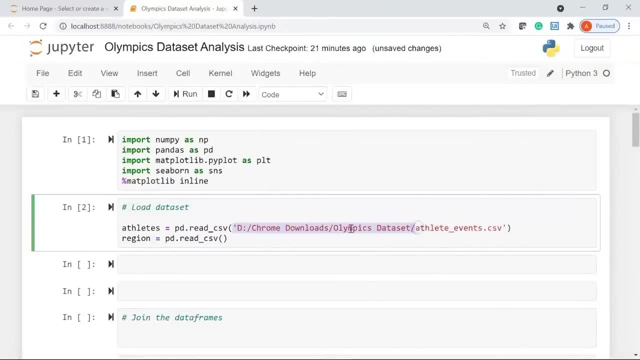 this file path till here, paste it and i will give my second file name, which is noc- underscore regions dot csv. you can verify here: the first one is athlete underscore events, the second one is noc- underscore regions. okay, i will close the quotation and we will run it again. 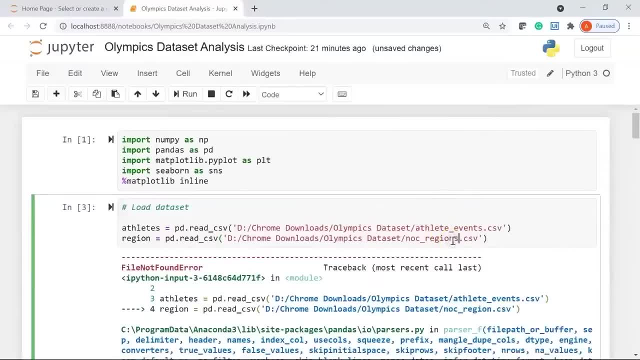 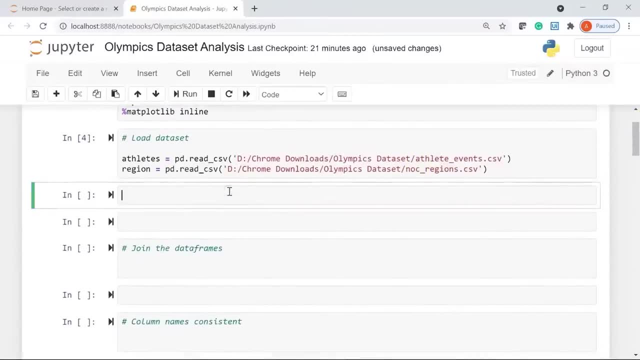 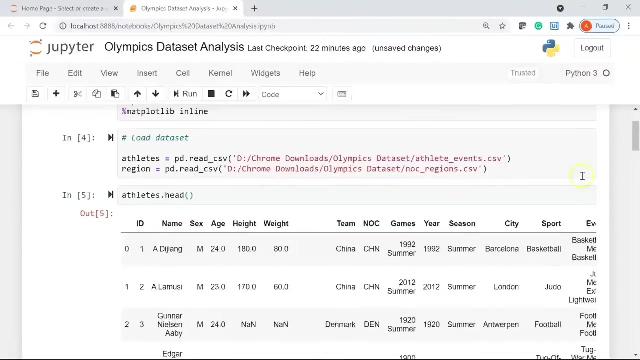 okay, there seems to be some error. i think this is regions, cool. now moving ahead, let's see the first few rows of both the data sets. i will use the head function for that. i will say athletes dot head. so this will print the first five rows from my data set. 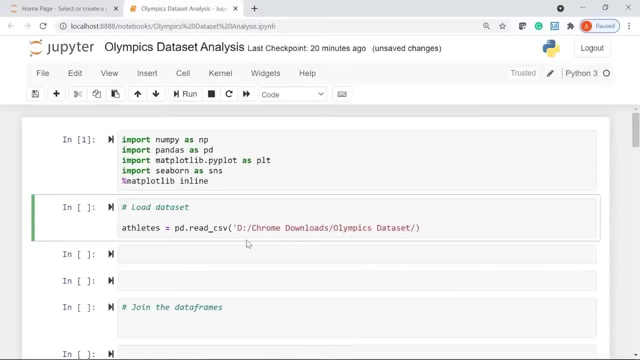 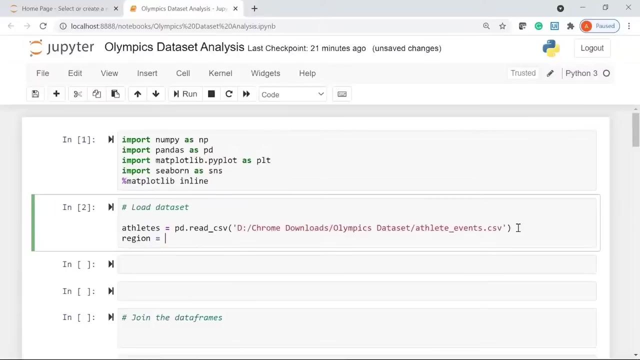 give another forward slash and after that i will give the file name, that is, athlete underscore- events dot csv. i will close the quotation. let's run it ok. similarly, we will load this second dataset. i will create another variable called regions, so it will have my data frame. i will use the same. 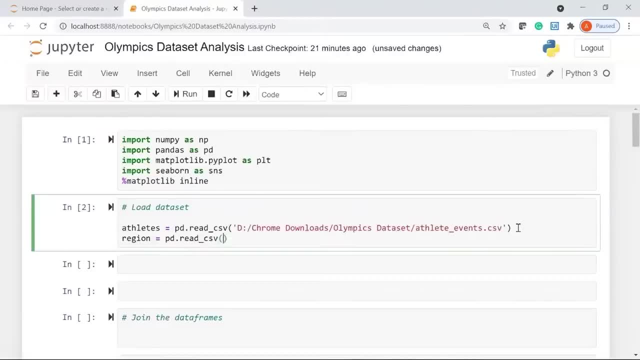 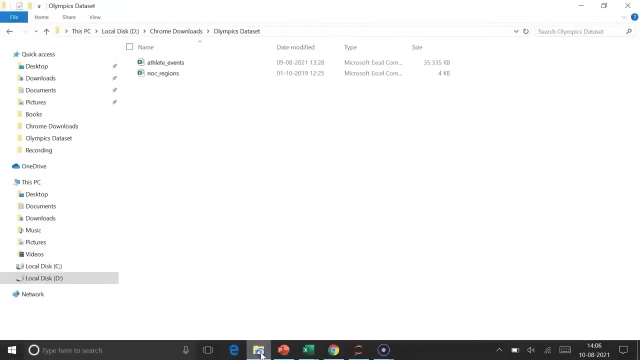 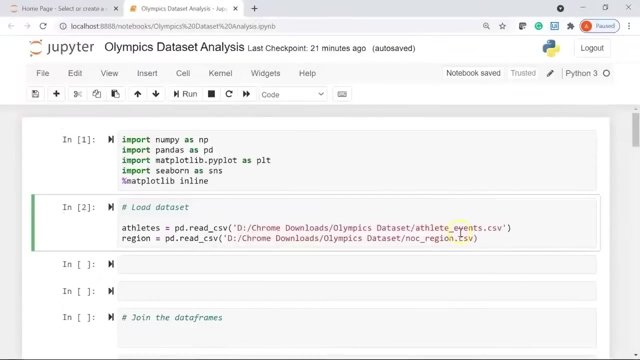 function pd dot read underscore csv. i will just copy this file path till here, paste it and i will give my second file name, which is noc- underscore regions dot csv. you can verify here: the first one is athlete underscore events, the second one is noc- underscore regions. ok, 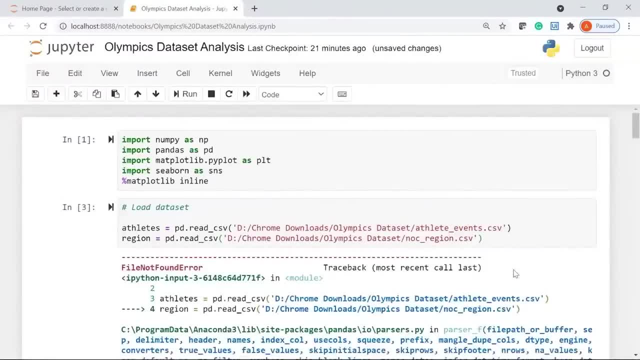 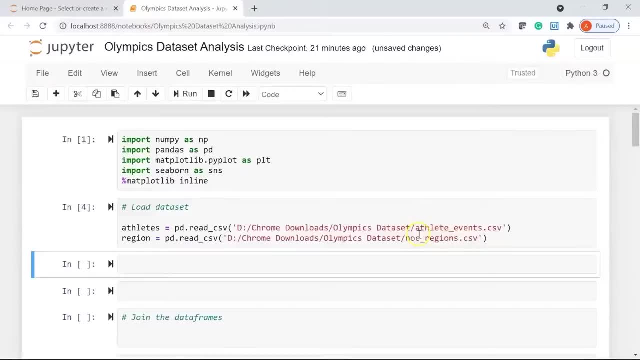 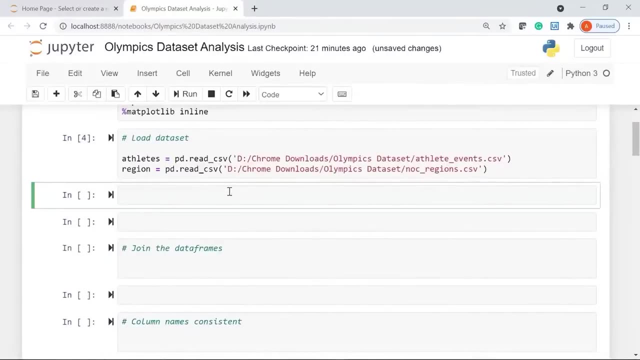 i will close the quotation and will run it again. ok, there seems to be some error. i think this is regions- cool. now, moving ahead, let's see the first few rows of both the datasets. i will use the head function for that. i will say athletes dot head. 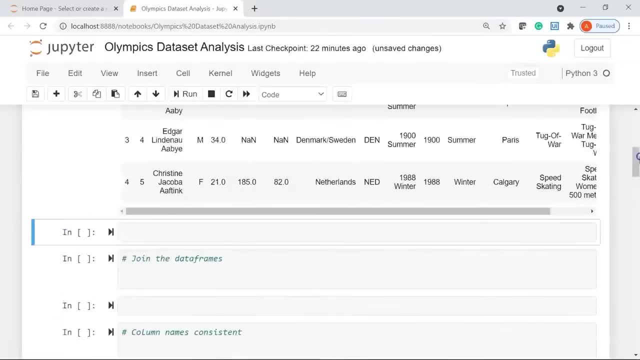 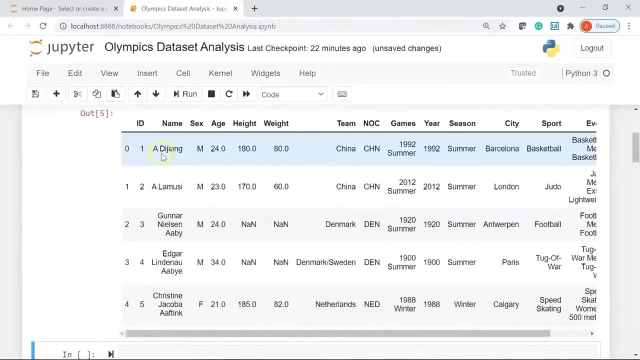 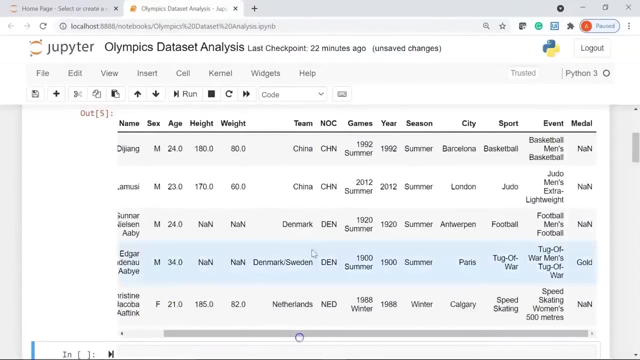 so this will print the first five rows from my dataset athletes. you can see here, from zero to four you have five rows of information: the id name, sex or the gender, age, height, weight. if i go to the right, you have games, year, season, sport event and medal. 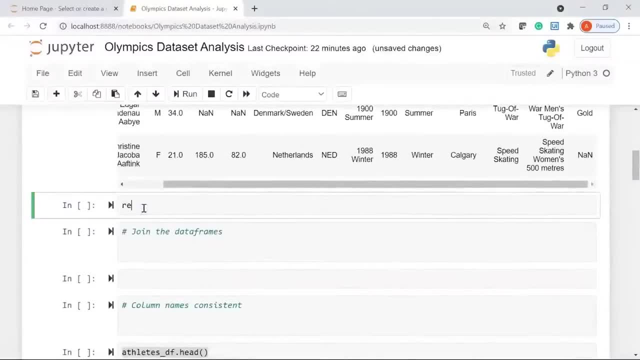 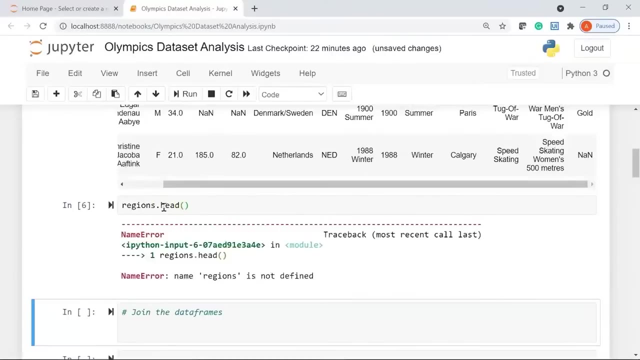 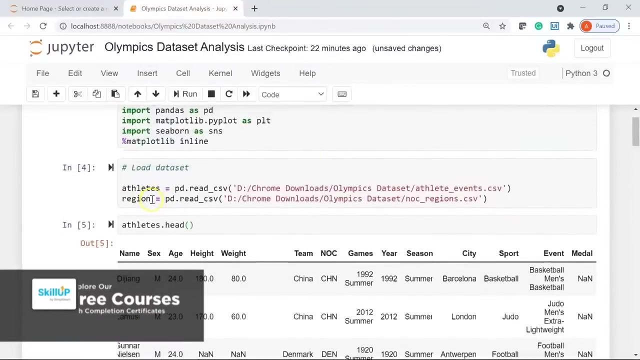 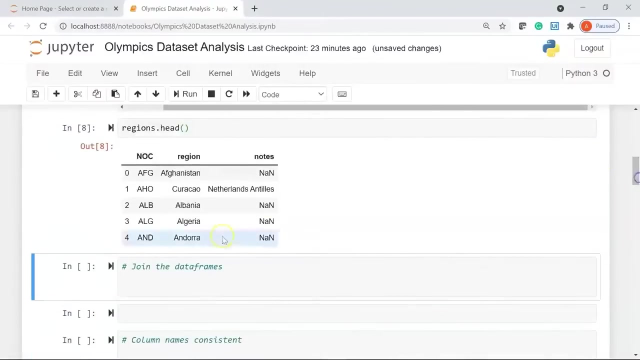 now let's see the second dataset that we imported, or loaded. i will say regions, dot head, and it says regions is not defined. let me cross check it. ok, i have taken it as region. let's make it regions cool now let's run it. there you go. so these are the 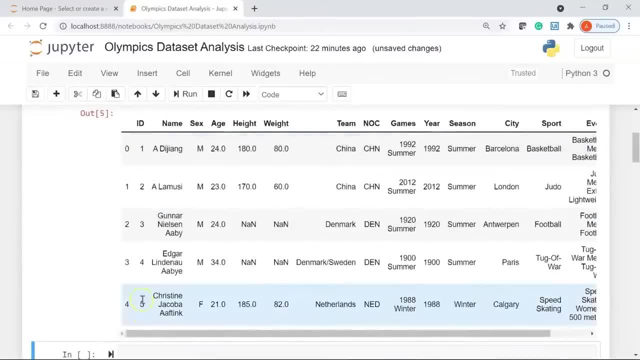 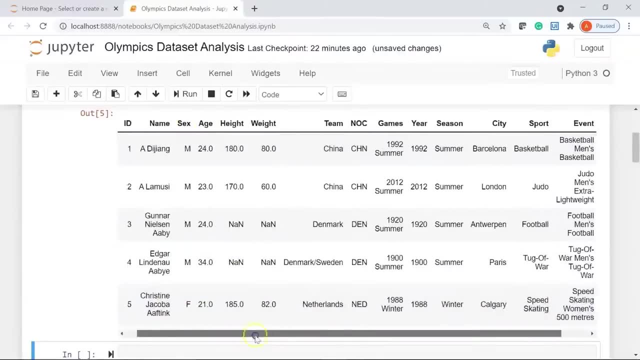 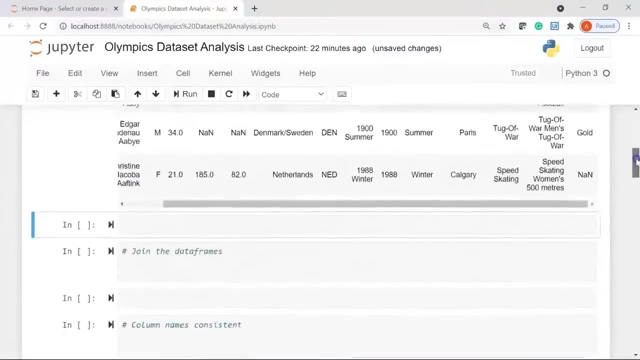 athletes. you can see here, from zero to four. you have five rows of information: the id name, sex or the gender, age, height, weight. if i go to the right, you have games, year, season, sport event and medal. now let's see the second data set that we imported. 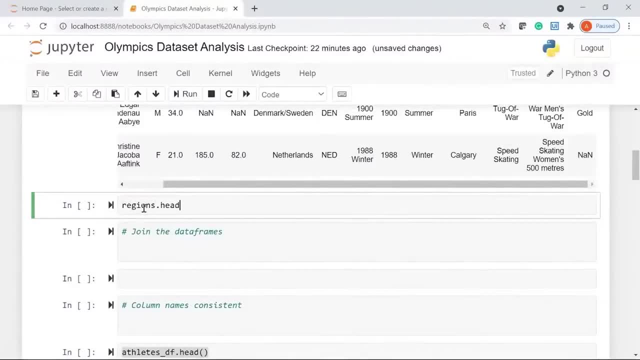 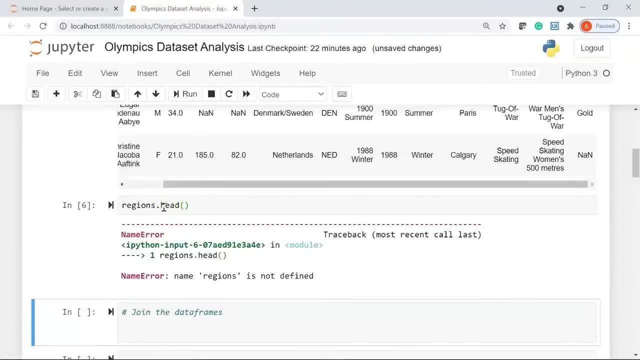 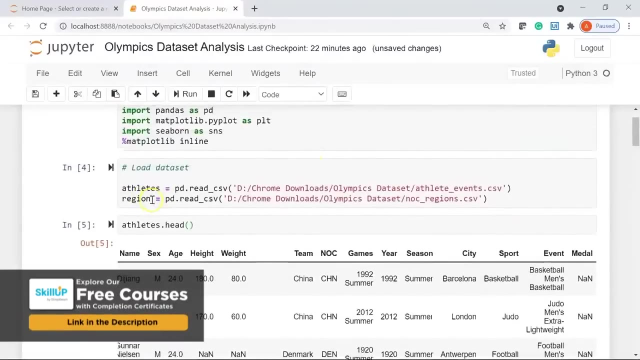 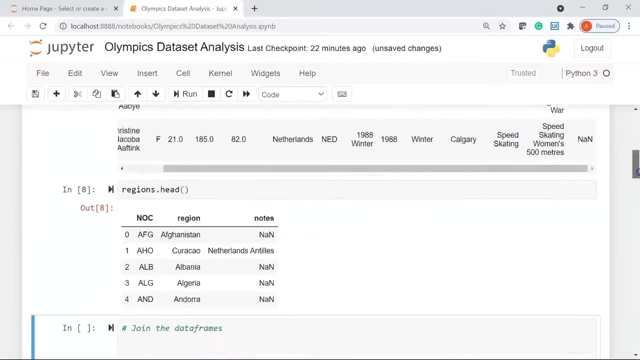 or loaded. i'll say regions dot head. it says regions is not defined. let me cross check it. okay, i have taken it as region. let's make it regions. cool, now let's run it. there you go. so these are the first five rows from our second data set. 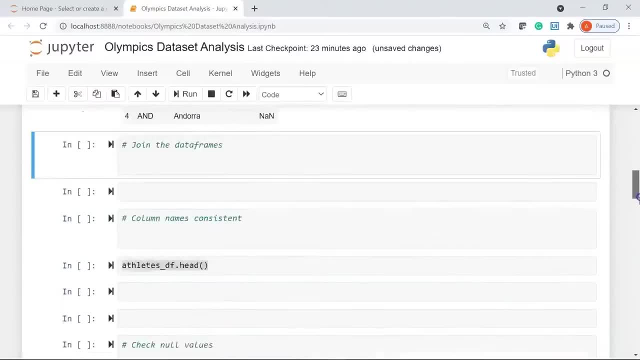 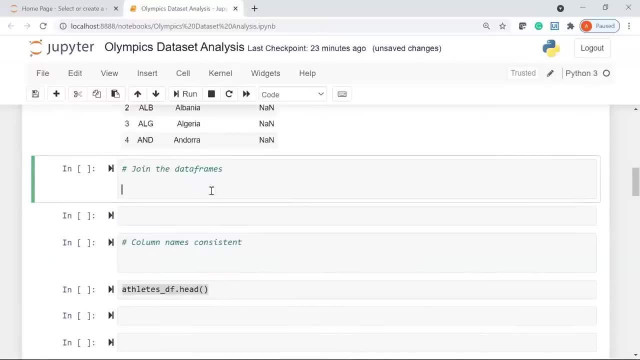 you have noc region and some nodes, alright. now the next step is to combine both the data sets. so we'll join the data frames using the pandas merge function. let me show you how to do it. so this is going to be a horizontal join. i'll create a variable. 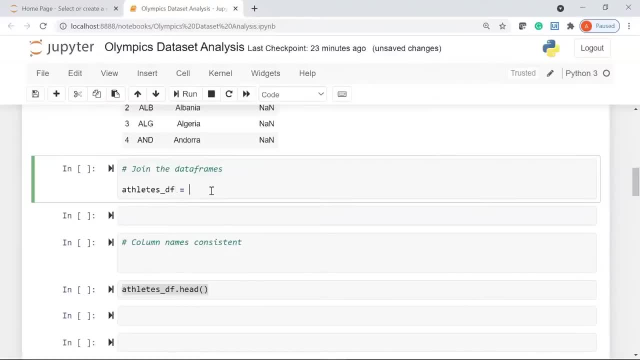 called athletes, underscore tf, then i'll use my first variable, which is athletes. i'll say dot merge, which is my function name. i'm going to merge the regions data frame. i'll use the how parameter in how i'll give my value, as i want to do a left join. 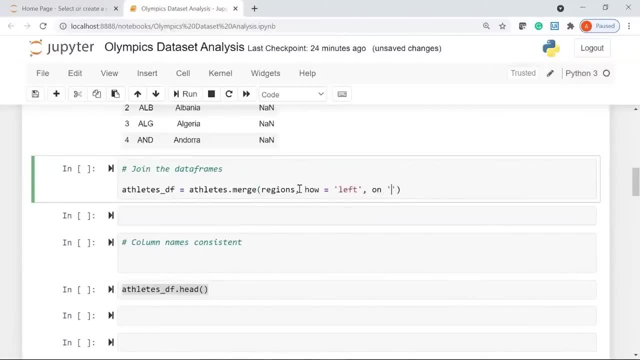 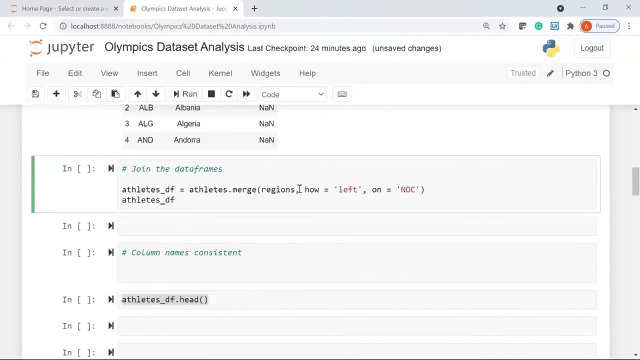 and my common column in both the data sets is actually noc. so i'm going to use the noc column as my common column to merge both the data sets. now let's go ahead and print the merged data frame. i'll say athletes, underscore: df, dot, head. let's run. 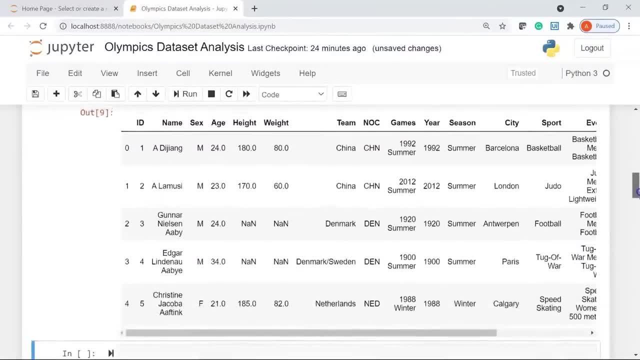 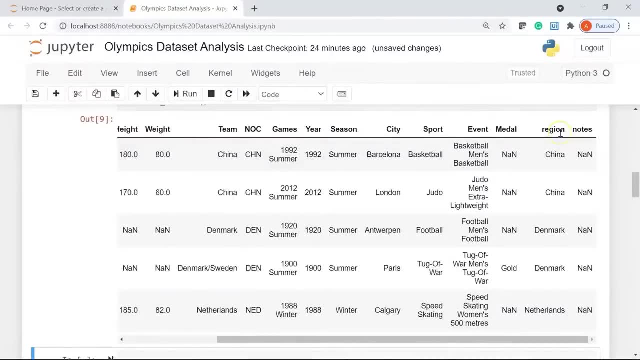 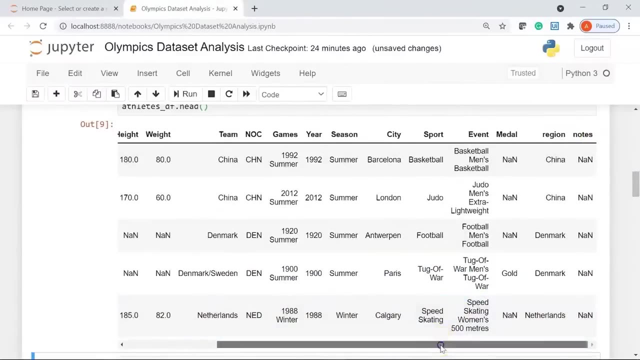 it. there you go. so, if you see clearly, if i move to the right, you can see here we have added two more columns that were present in the second data set, which was regions. so we have regions and nodes added to my first data set, that is, athletes. 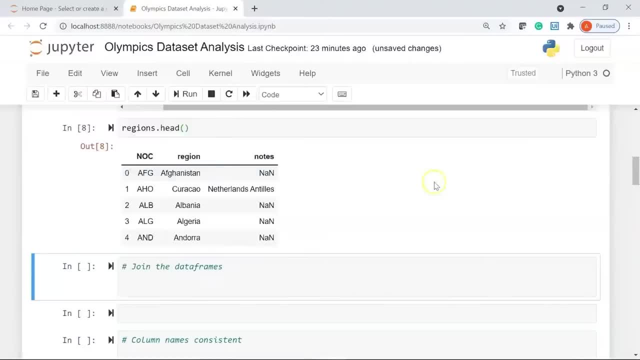 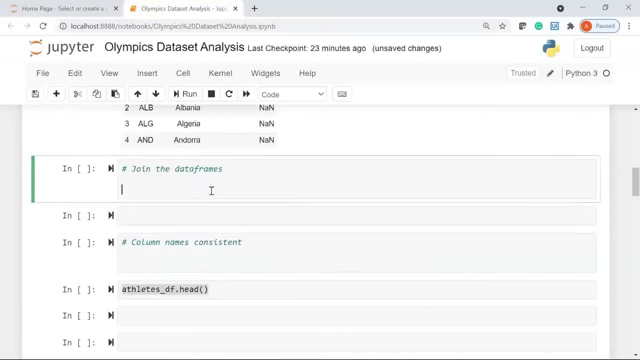 first five rows from our second dataset. you have noc, region and some nodes. alright, now the next step is to combine both the datasets. so we will join the data frames using the pandas merge function. let me show you how to do it. so this is going to be a horizontal join. 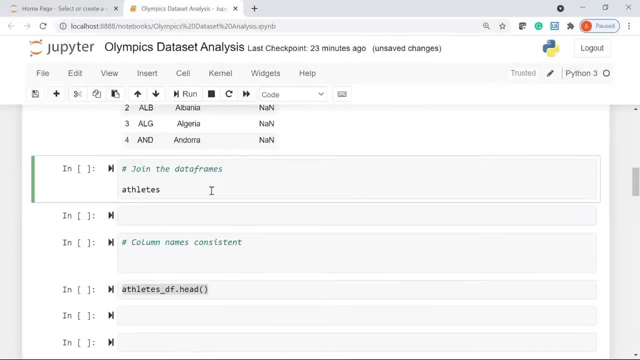 i will create a variable called athletes, underscore tf. then i will use my first variable, which is athletes. i will say dot merge, which is my function name. i am going to merge the regions data frame. i will use the how parameter in how i will give my value as. 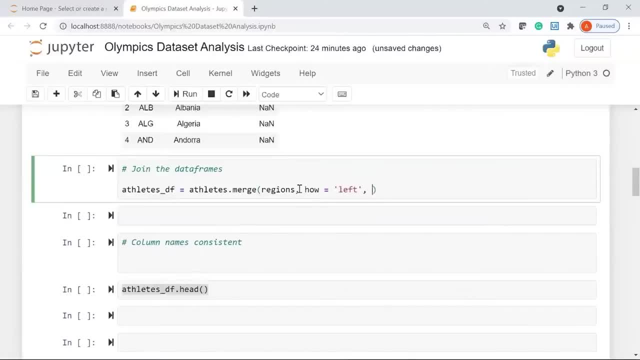 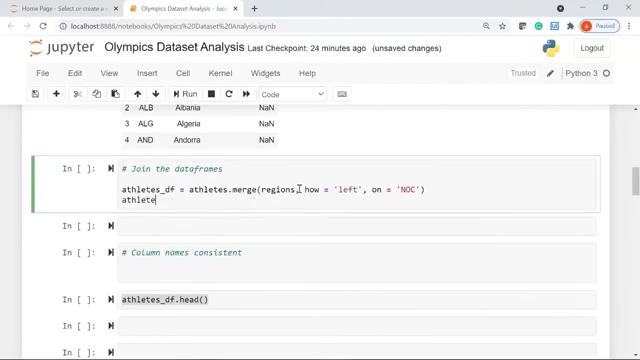 i want to do a left join and my common column in both the datasets is actually noc. so i am going to use the noc column as my common column to merge both the datasets. now let's go ahead and print the merged data frame. i will say athletes. 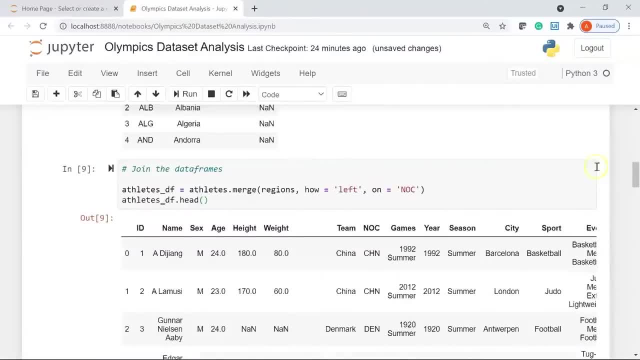 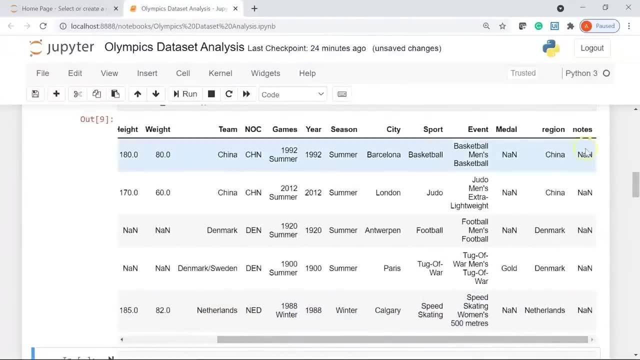 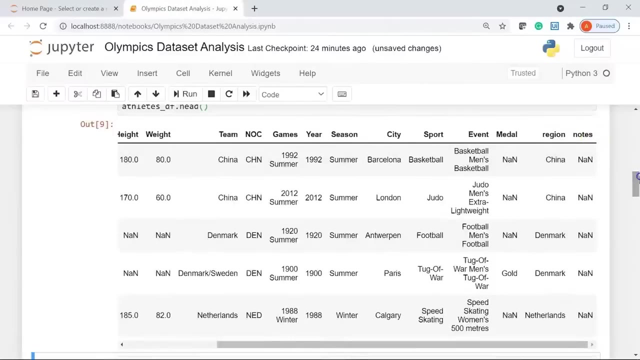 underscore: df dot head. let's run it. there you go. so, if you see clearly, if i move to the right, you can see here we have added two more columns that were present in the second dataset, which was regions. so we have regions and nodes added to my 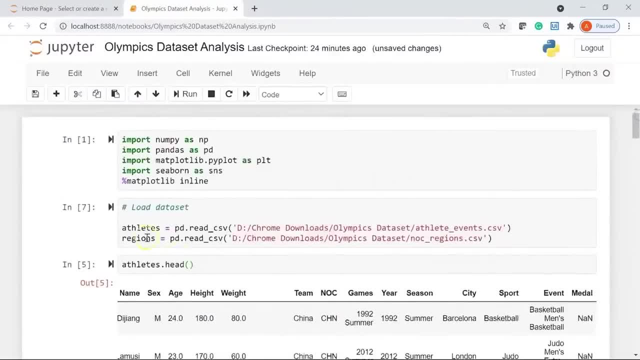 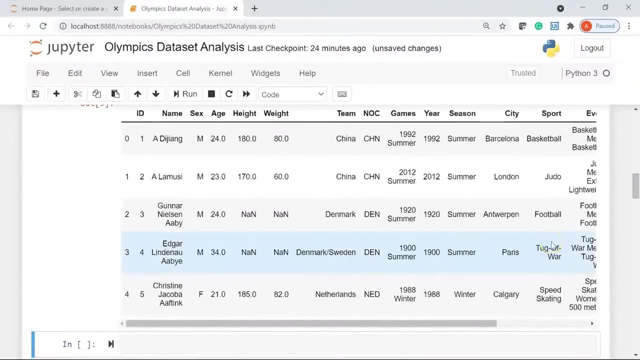 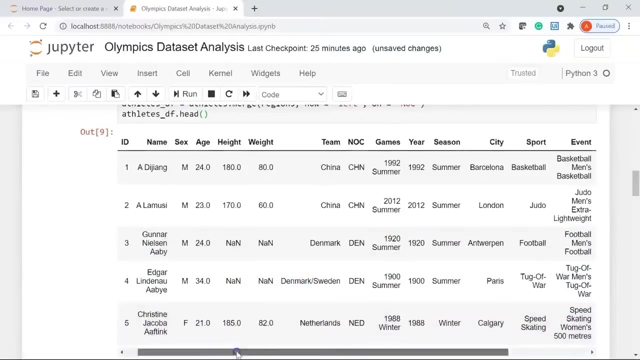 first dataset, that is, athletes underscore events- cool. now, one thing to note here is see, the column names are not consistent. if you see here, the rest of the columns start with a capital letter, but if you see the last two columns that we just added now start with a lower case letter. 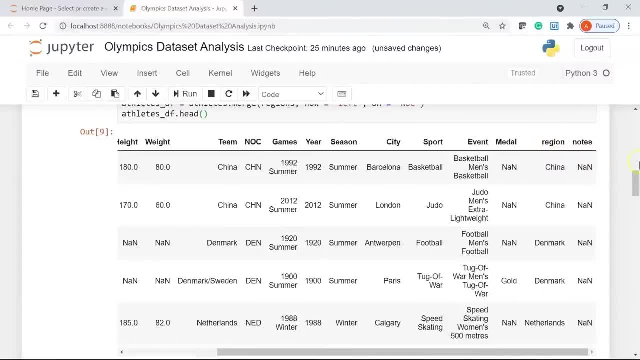 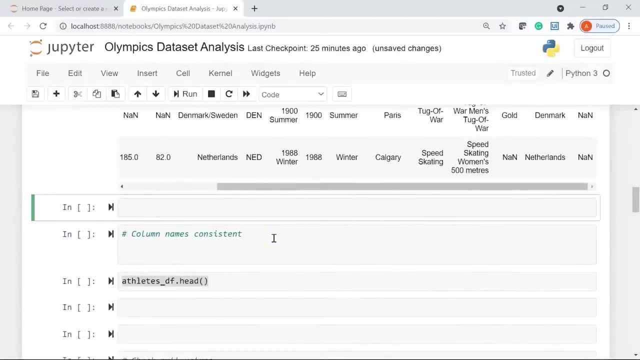 so we will use the rename function to make the column names consistent. but before that let's see the shape of the data frame. so i will print the shape of the data frame to know the total number of rows and columns. i will say athletes if i hit tab. 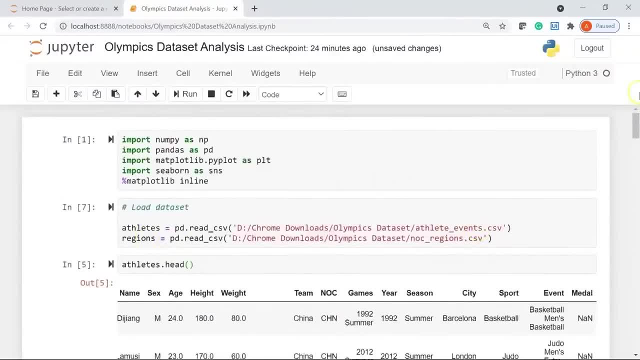 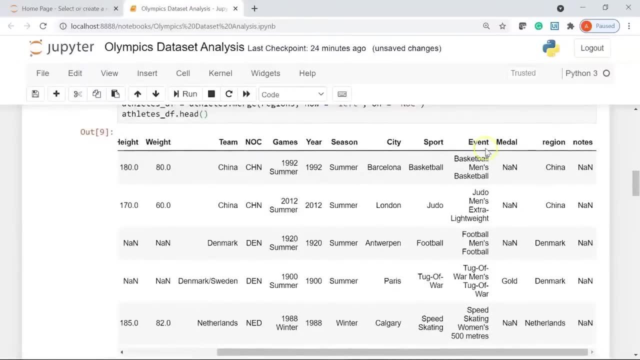 athletes underscore events- cool. now, one thing to note here is see, the column names are not consistent. if you see here, the rest of the columns start with a capital letter, but if you see, the last two columns that we just added now start with a lower case letter. so we'll 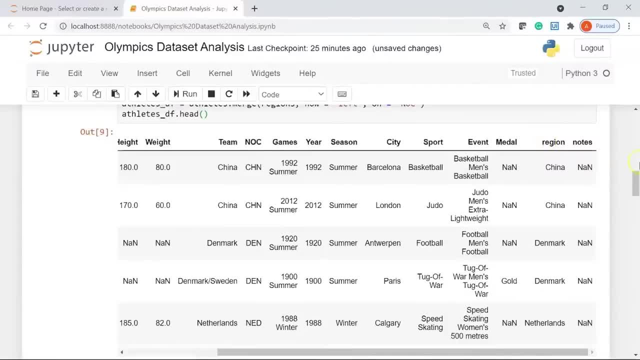 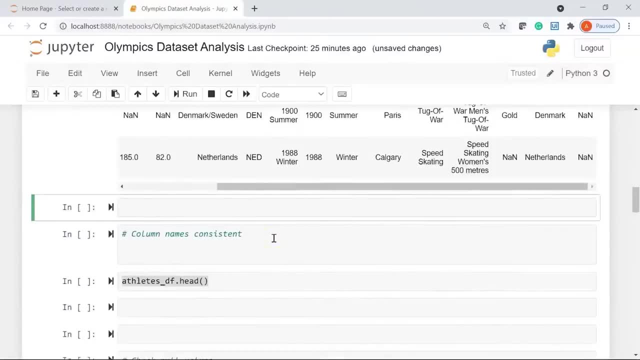 use the rename function to make the column names consistent. but before that let's see the shape of the data frame. so i'll print the shape of the data frame to know the total number of rows and columns. i'll say athletes. if i hit tab, you'll see. it will give me. 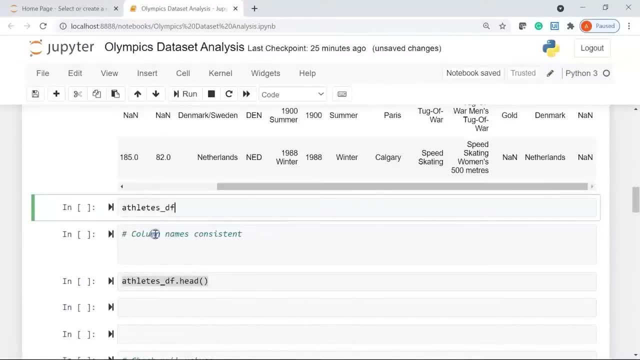 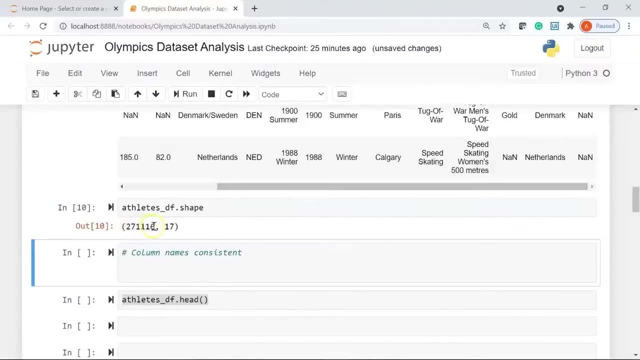 the prompt. i'll select athletes underscore df. i'll use the shape attribute. let's run it and see the result. you can see here. it gave me the total number of rows, so 271116 rows, and earlier we had 15 columns in the first data set, and now that we have added, 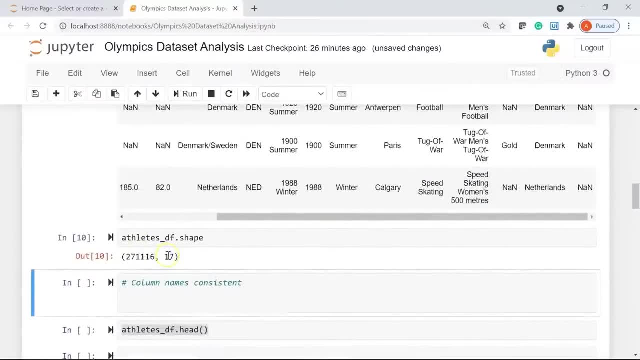 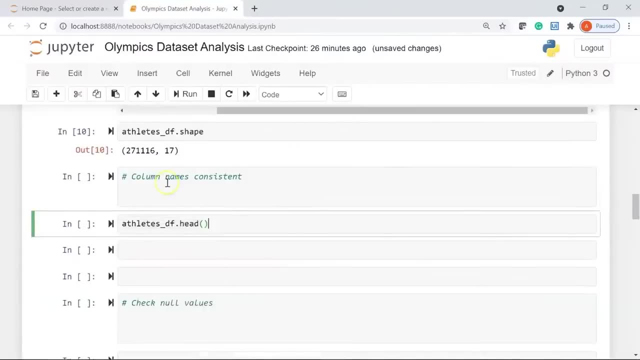 two more columns, so the total number of columns becomes 17. now, cool. so now it's time to make the column names consistent. so i'll show you how to do it. i'll say athletes- underscore, df, dot. i'll use the rename function and then i'll 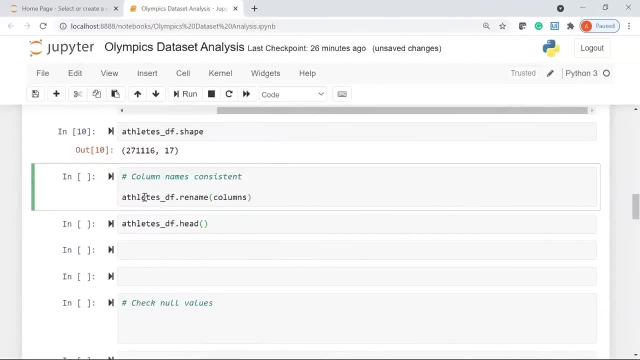 say columns equal to, i'll use curly braces. my first column, that is region. i want to change it to a region, but the r should be capital now, or upper case. give a comma and then say: my second column, this should be a region actually. my second column, that is notes. 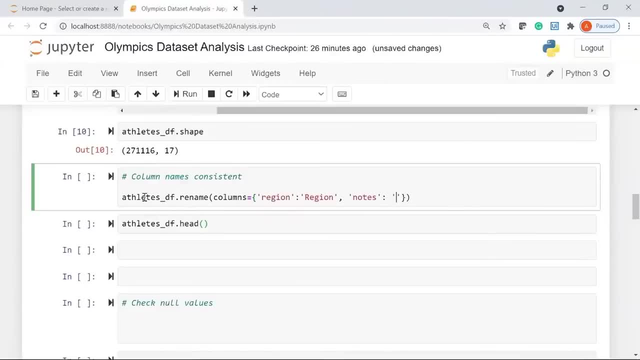 i want to change the first letter to upper case, so i'll say capital n. the rest all remains same. we'll give a comma here and say in place equal to true. so it will change the column names and will reflect in this. athletes underscore: df data frame. 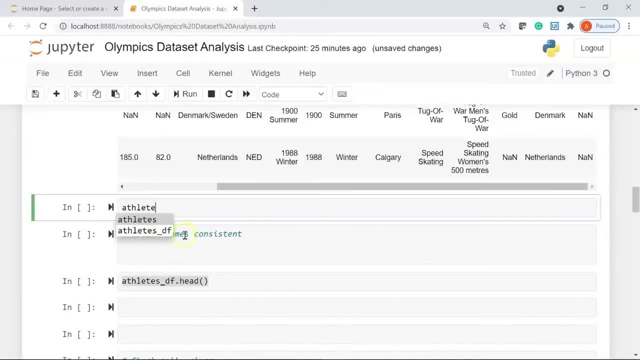 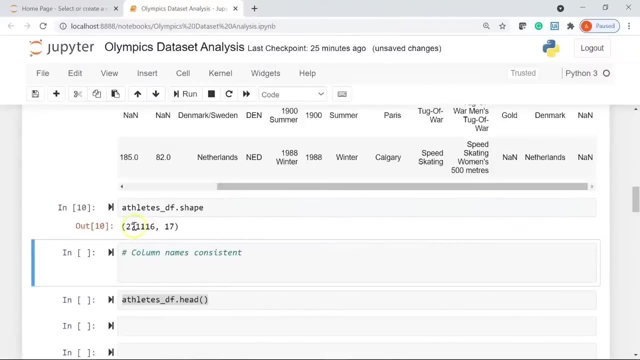 you will see. it will give me the prompt. i will select athletes underscore df. i will use the shape attribute. let's run it and see the result. you can see here. it gives me the total number of rows, so 271116 rows, and earlier we had 15 columns in the 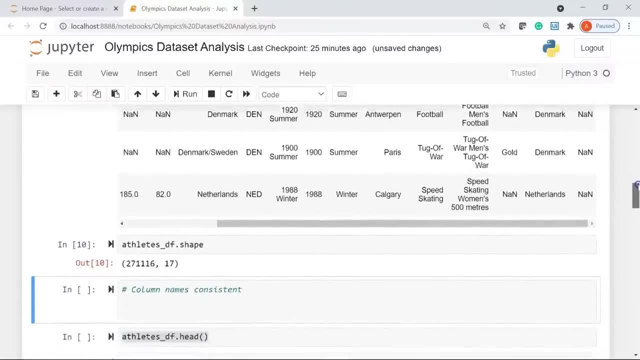 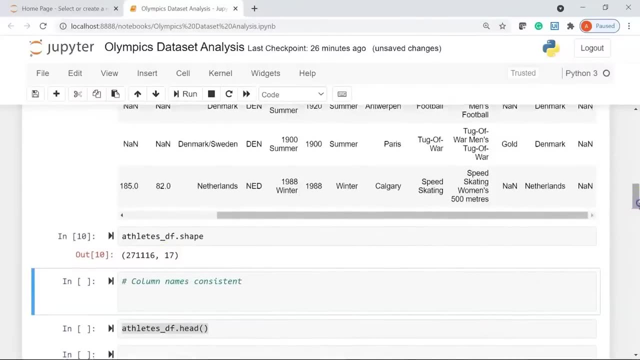 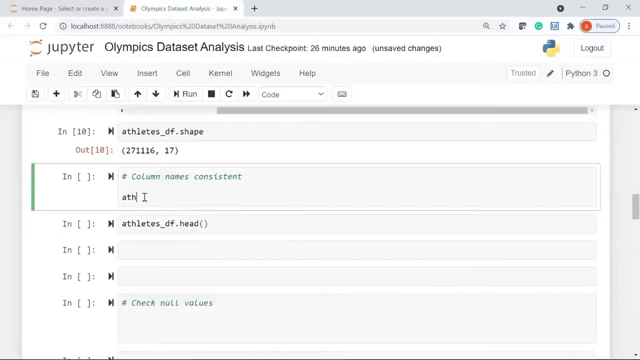 first dataset, and now that we have added two more columns, so the total number of columns becomes 17. now, cool. so now it's time to make the column names consistent. so i will show you how to do it. i will say athletes, underscore df, dot. i will use the rename function. 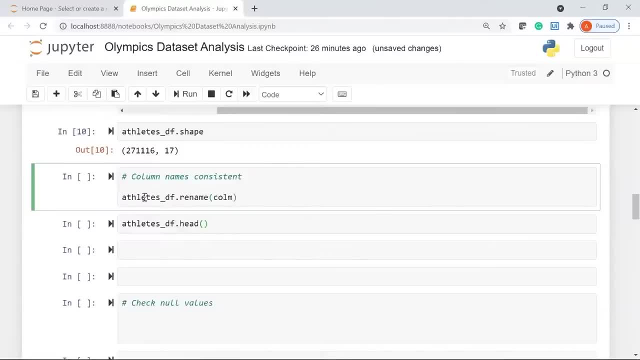 and then i will say columns equal to. i will use curly braces: my first column, that is region. i want to change it to region, but the r should be capital now, or upper case. give a comma and then say: my second column, this should be region actually. and then 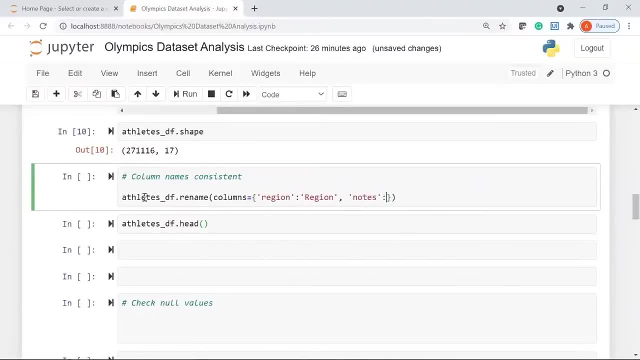 my second column, that is nodes. i want to change the first letter to upper case, so i will say capital n. the rest all remains same. i will give a comma here and say in place equal to true. so it will change the column names and will reflect in this athletes underscore. 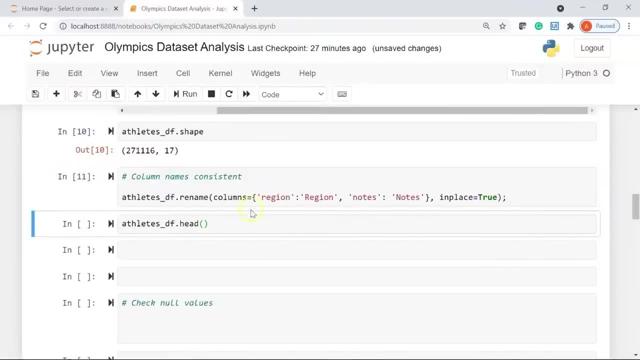 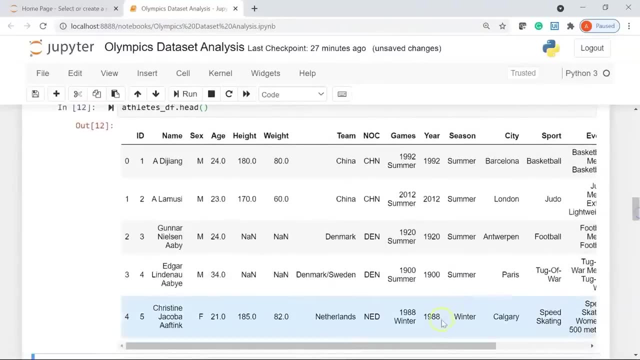 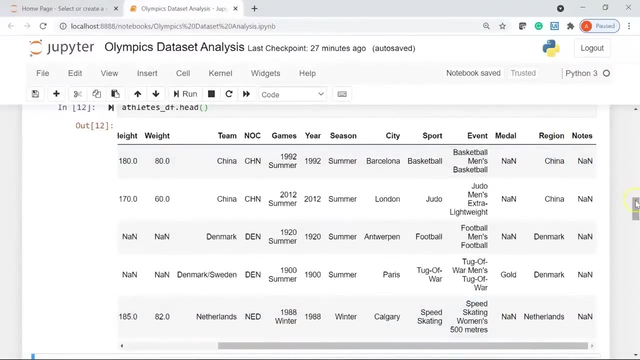 df data frame. let's run it now to verify. you can again use the head function. i will run this again. let me scroll down and move to the right. you can see the difference. there you go. so we have successfully renamed the last two columns: region and nodes. 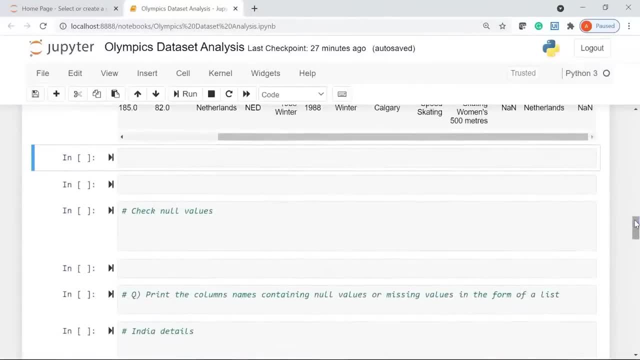 alright, now moving ahead. now i will show you how you can use the info method to print information about a data frame, including the index data type, the column data types, the nominal values and memory usage. so for that, you just need to use the info function, so i will write. 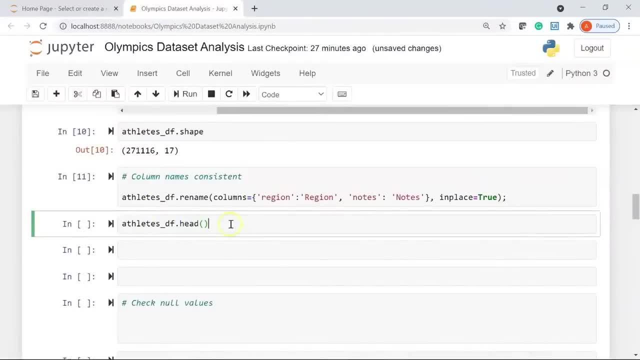 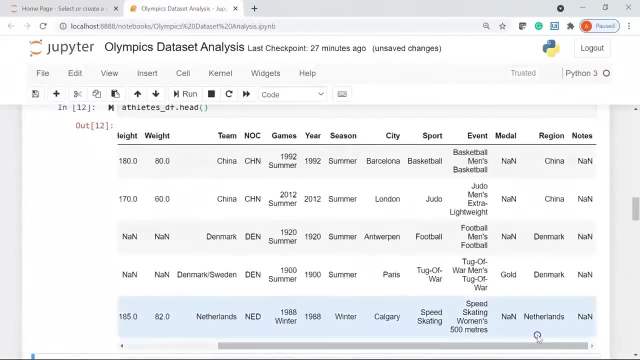 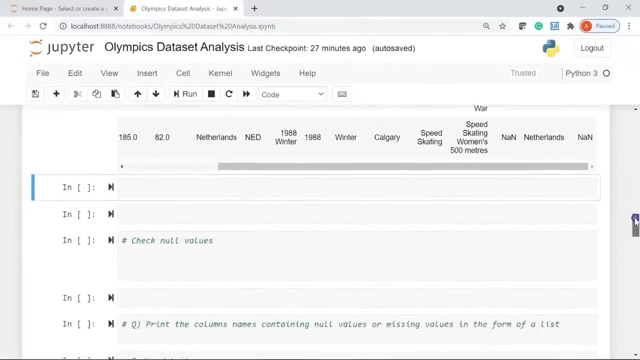 let's run it now to verify you can again use the head function. i'll run this again. let me scroll down and move to the right. you can see the difference. there you go. so we have successfully renamed the last two columns: region and notes. alright, now moving ahead. 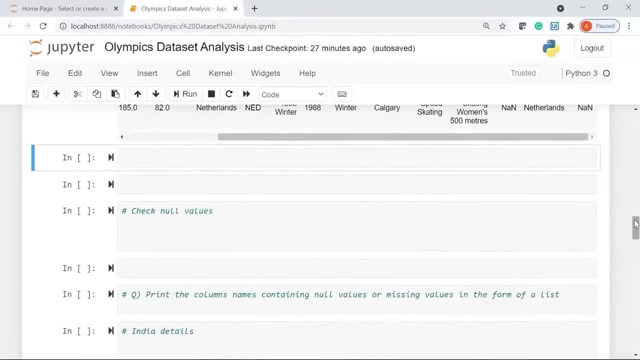 now i'll show you how you can use the info method to print information about a data frame, including the index data type, the column data types, non null values and memory usage. so for that you just need to use the info function. so i'll write athletes underscore df. 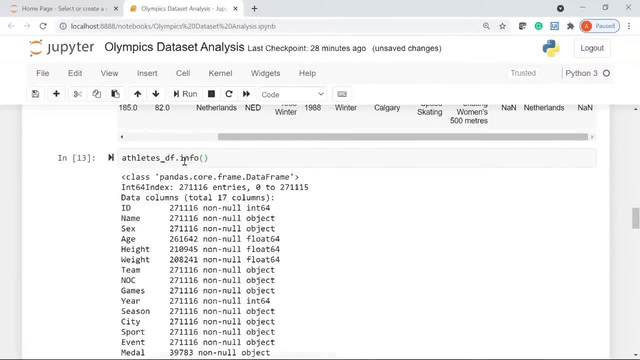 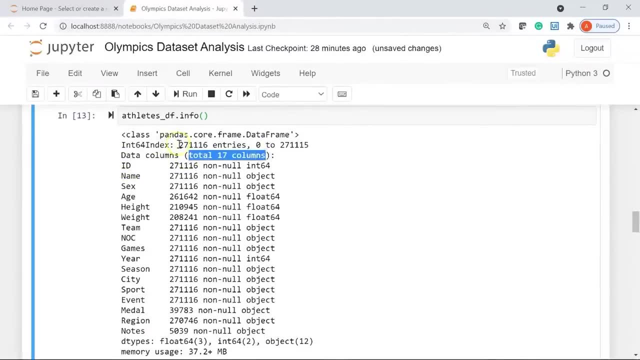 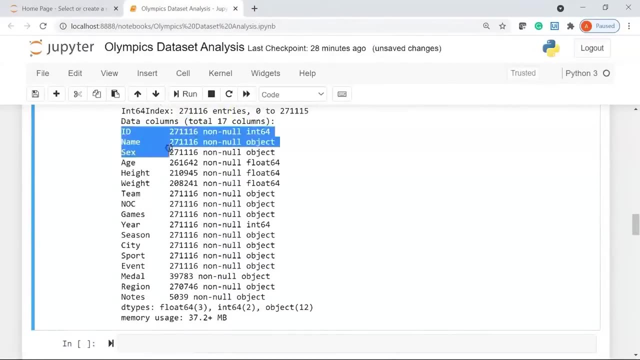 dot info. let's run it. there you go. so here we have the data columns. you can see total 17 columns. you have 271116 rows or entries. then you have the different column names and it says non null and the data type of the column. below you can see some information. 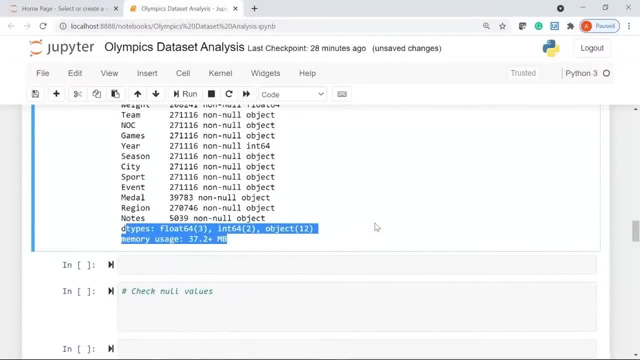 about the memory usage, alright. next, the describe method is used for calculating statistical information, such as mean, standard deviation, the percentiles of the numerical values of the data frame and much more. it analyzes both numeric and object series and also the data frame column sets of mixed data types. 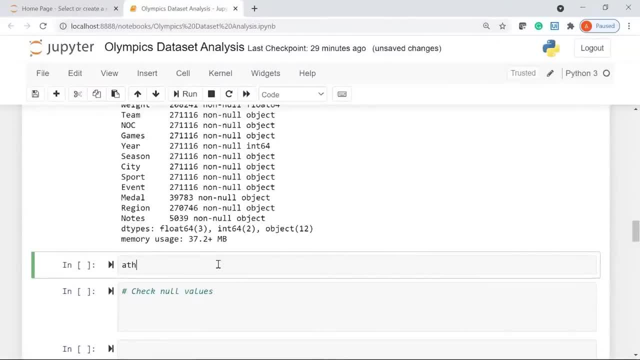 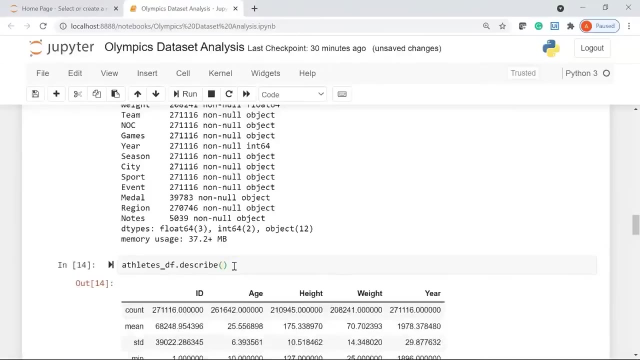 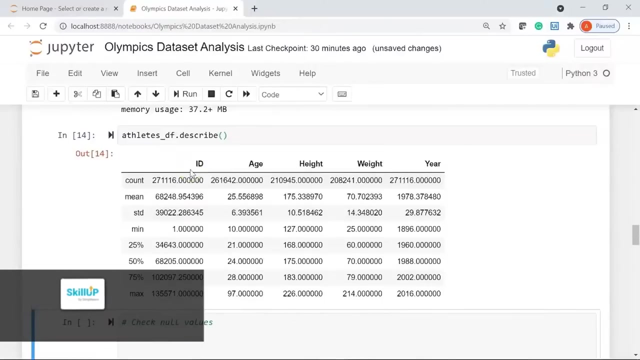 so let me show you how, using the describe function, you can display some statistical summary. i'll just write describe and give parenthesis. let's run it ok. if i scroll down, you can see here: by default the describe function will only give information about numerical columns. so here you can see we have the total count. 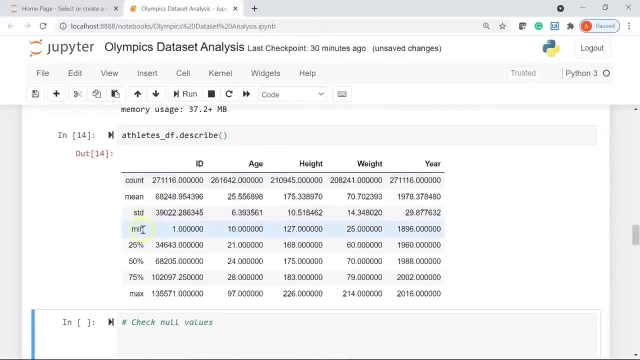 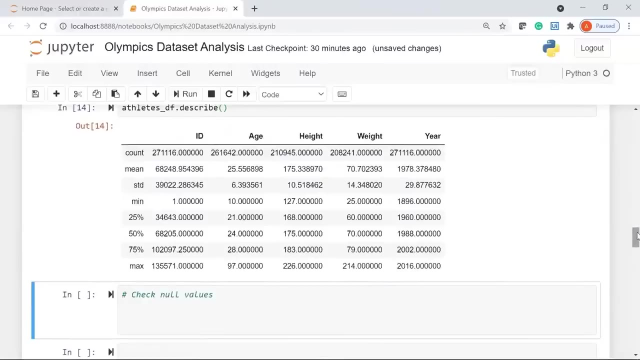 the mean of each of these columns. you have the standard deviation, the minimum and maximum value, and then we have the 25th percentile, the 50th percentile and the 75th percentile value of the columns: id, age, height, weight and year. alright, now one thing to notice. 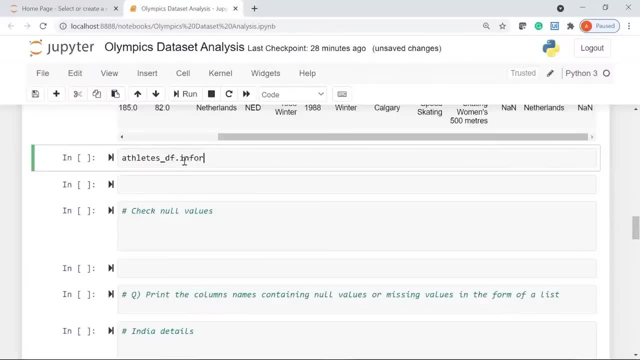 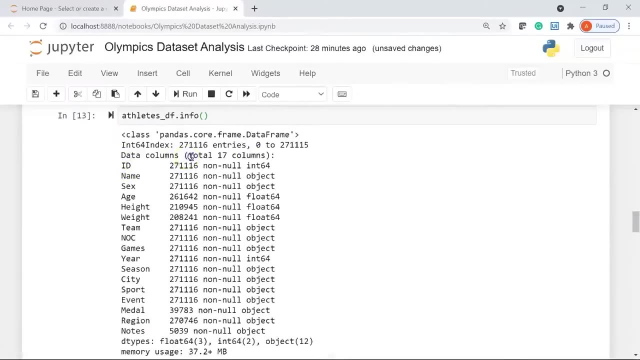 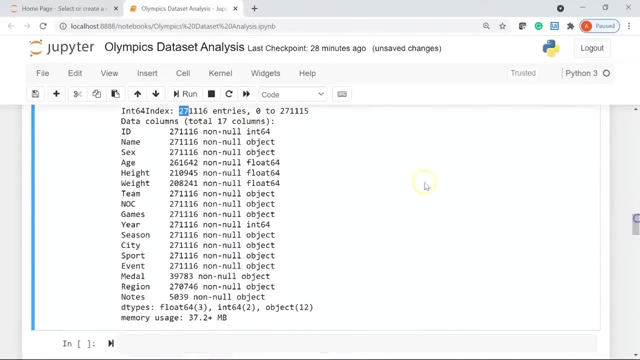 athletes: underscore: df dot info. let's run it, there you go. so here we have the data columns. you can see total 17 columns. you have 271116 rows or entries. then you have the different column themes and it says non null and the data type of the. 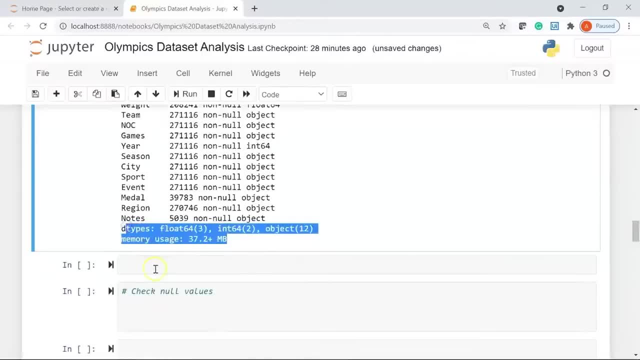 column below you can see some information about the memory usage, alright. next, the describe method is used for calculating statistical information such as mean, standard deviation, the percentiles of the numerical values of the data frame and much more. it analyzes both numeric and object series, and also the 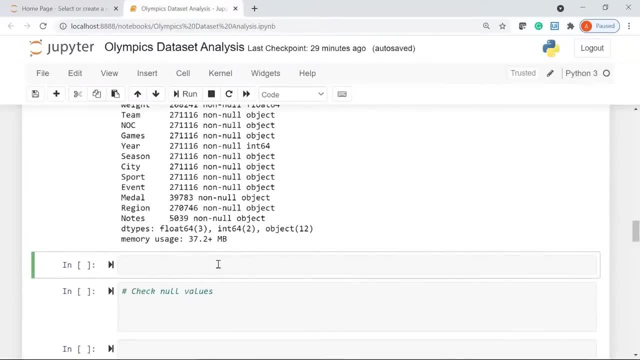 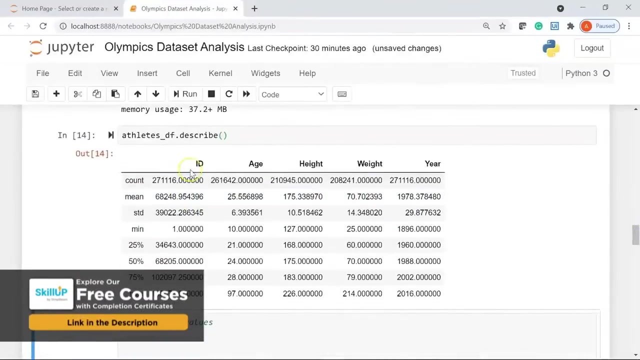 data frame column sets of mixed data types. so let me show you how, using the describe function, you can display some statistical summary. i will just write describe and give parenthesis. let's run it. ok. if i scroll down, you can see here: by default, the describe function will only give information. 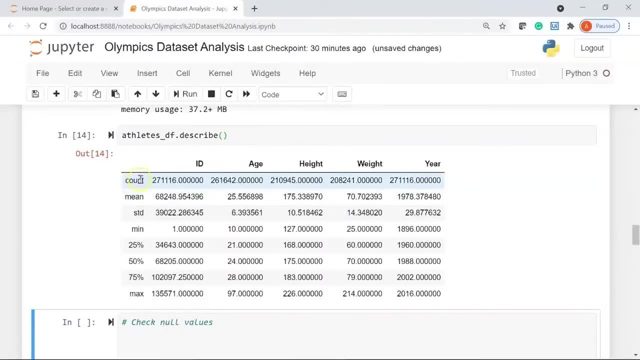 about numerical columns. so here you can see. we have the total count, the mean of each of these columns, you have the standard deviation, the minimum and maximum value, and then we have the 25th percentile, the 50th percentile and the 75th percentile value of. 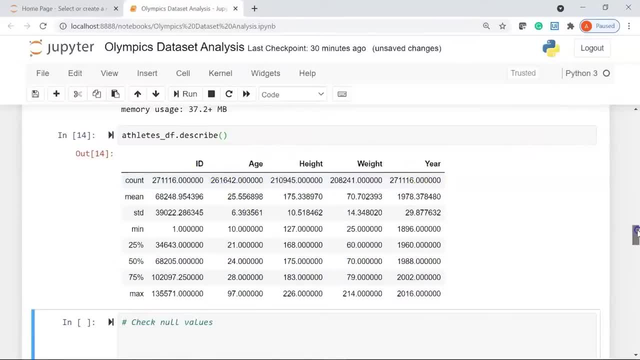 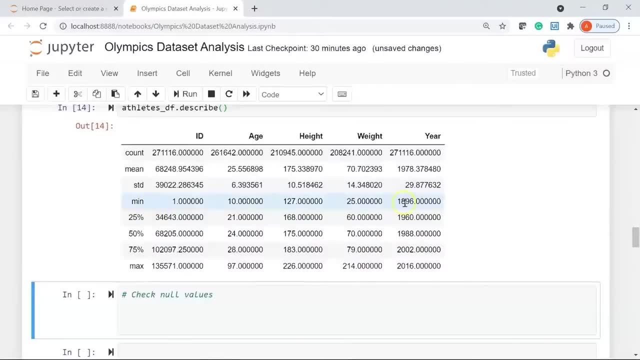 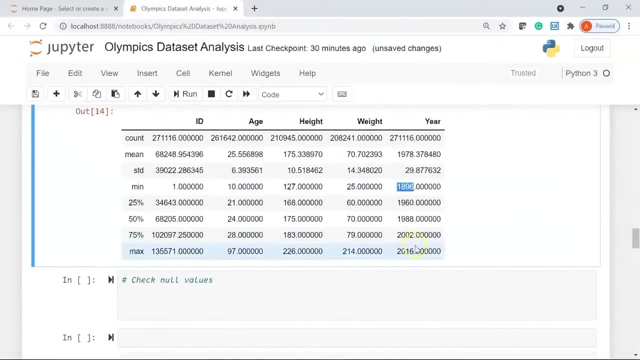 the columns: id, age, height, weight and year. alright, now one thing to notice here is, if you see the year column, the minimum year is 1896, so this is when olympics started and, until recently, the rio olympics that was held in 2016. 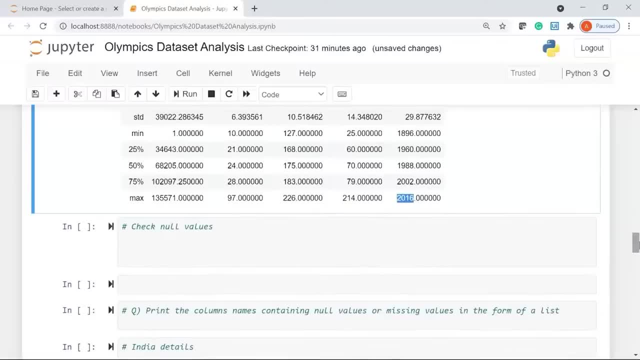 alright, now moving ahead. now let's check if there are any null values present in the columns of the data set. so first i am going to create a variable called nan values give equal to, i will say, athletes, underscore df, and the function to check is, i will say, is any? 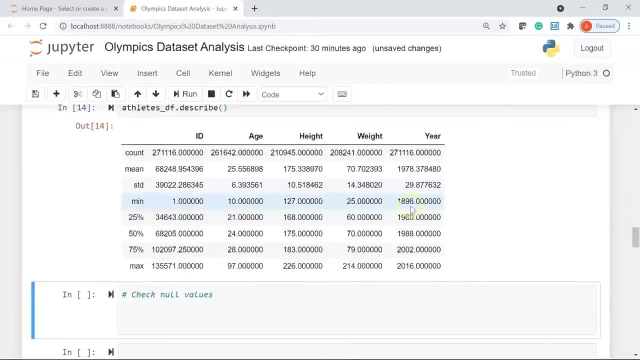 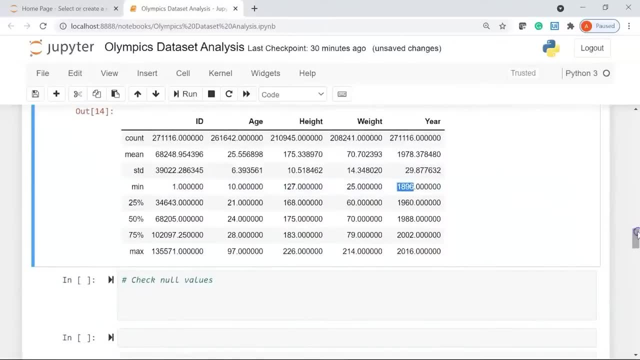 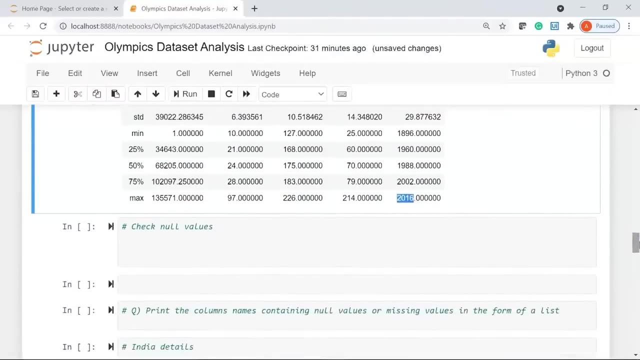 here is, if you see the year column, the minimum year is 1896, so this is when olympics started and, until recently, the rio olympics that was held in 2016. alright, now moving ahead. now let's check if there are any null values present. 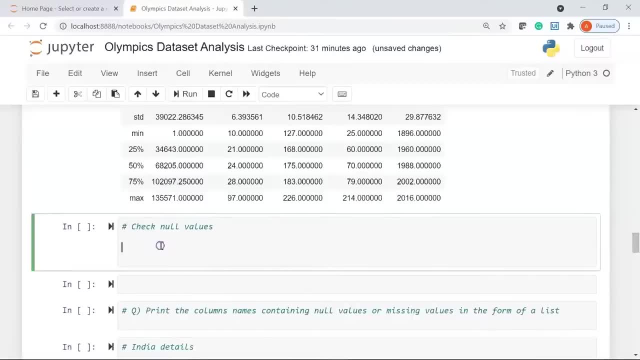 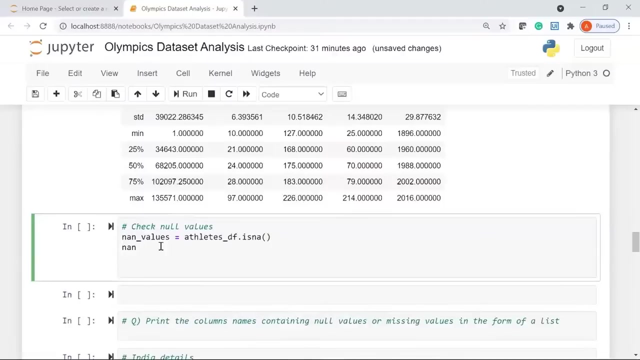 in the columns of the data set. so first i am going to create a variable called nan values give equal to, i will say, athletes, underscore df, and the function to check is, i will say: is any. i will create another variable called nan underscore columns, and here i will use the 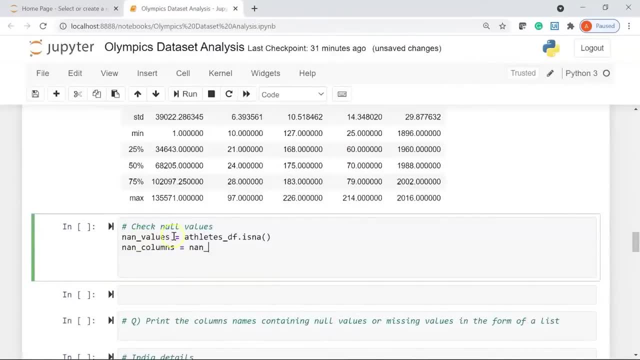 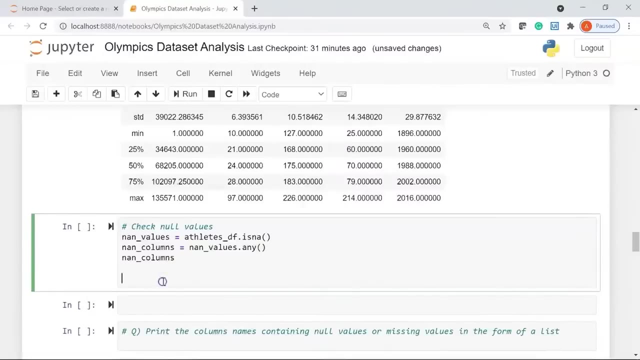 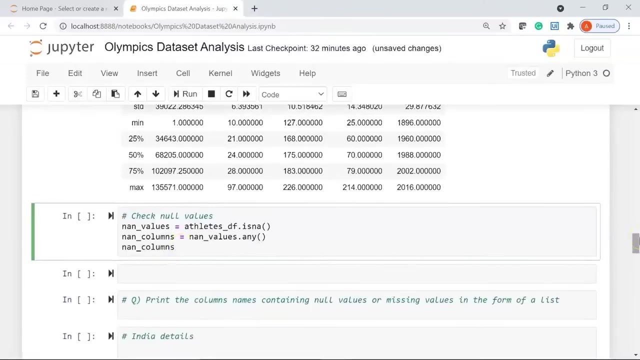 any function, i will say nan. underscore this variable, which is underscore values dot. i will say any and i will print my nan columns variable so this will display the result in terms of boolean values. so if there are any null or nan or missing values in any of 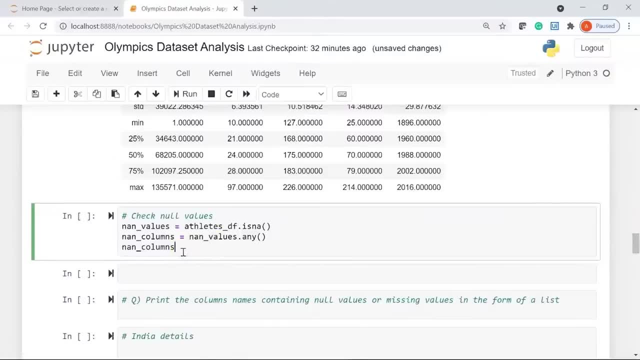 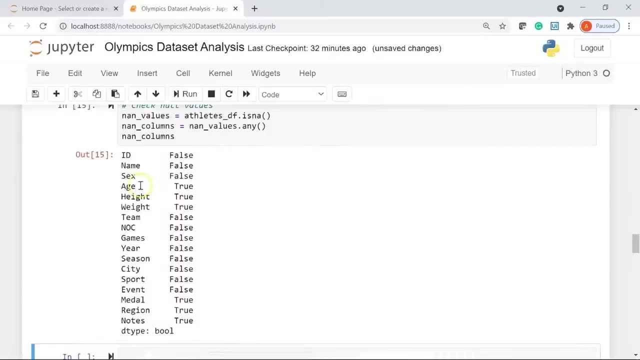 the columns, it will say true, otherwise it will say false. let's display the result. there you go. so if you mark here clearly: so there are nearly six columns where we have missing values. you have age, height, weight, medal region and notes- columns that have missing values. so hence, 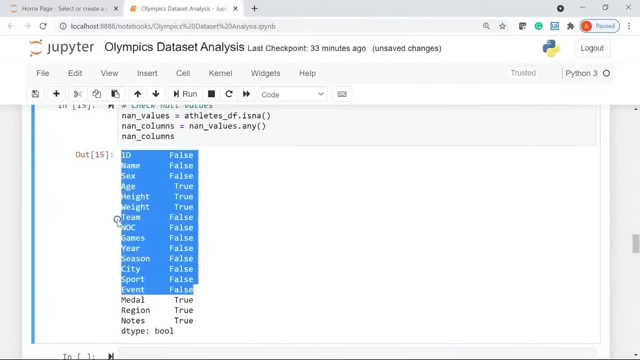 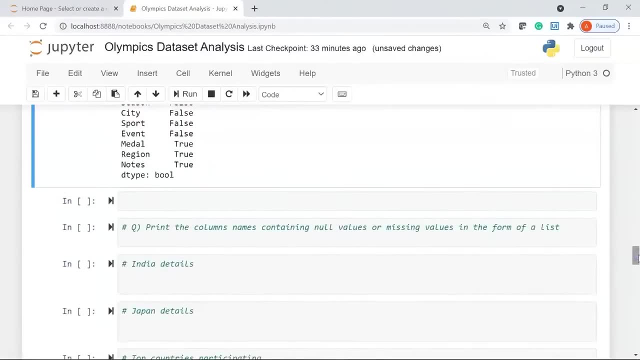 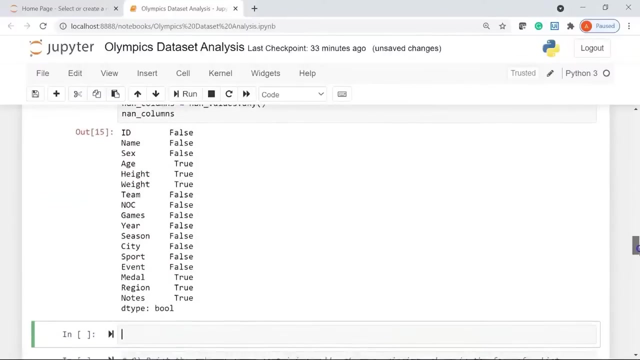 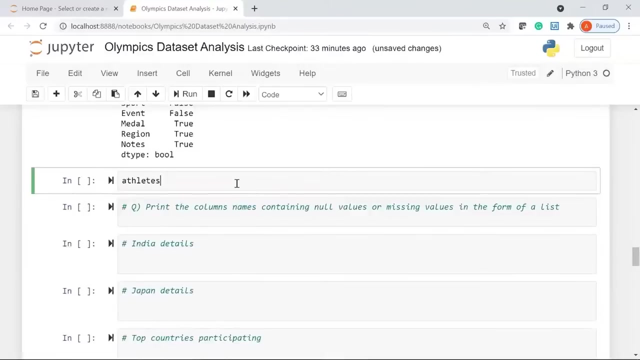 it has given us. true, the rest of the columns do not have any nan or missing values, hence they are false. alright, let me scroll down. now. let's see the total number of null values for the above six columns. so i will say athletes, underscore: df, dot. i will use the function. 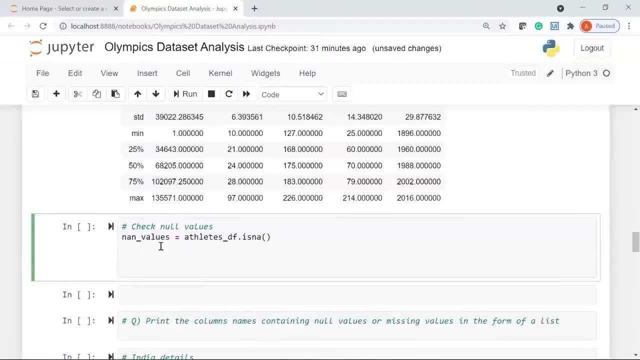 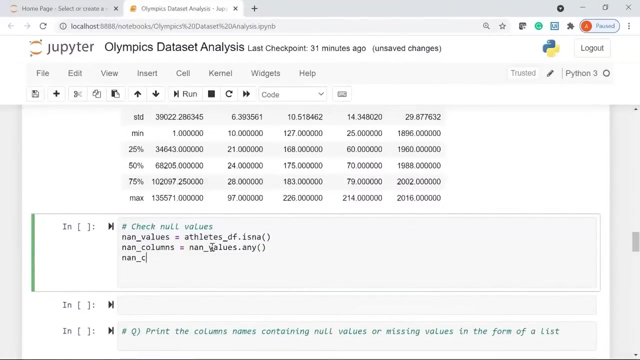 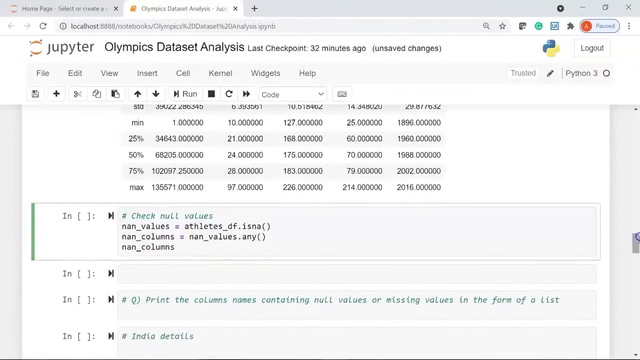 i will create another variable called nan underscore columns, and here i will use the any function. i will say nan underscore this variable, which is underscore values dot, i will say any and i will print my nan columns variable. so this will display the result in terms of boolean values. 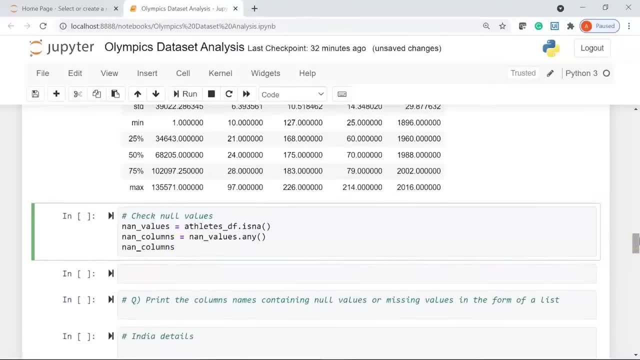 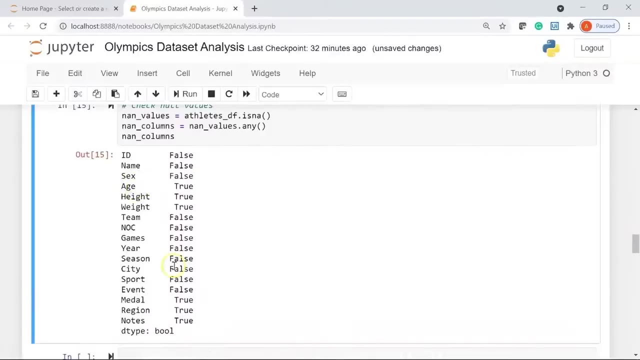 so if there are any null or nan or missing values in any of the columns, it will say true, otherwise it will say false. let's display the result there you go. so if you mark here clearly, so there are nearly six columns where we have missing values. we have age, height, weight. 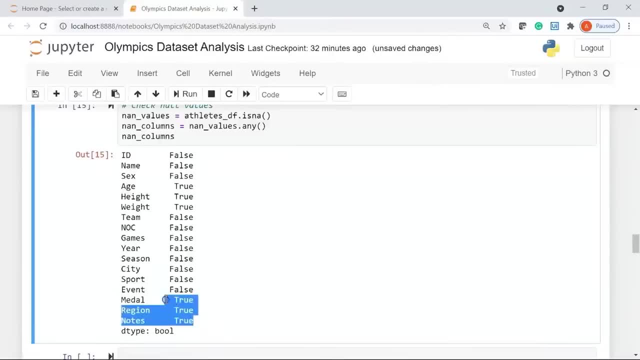 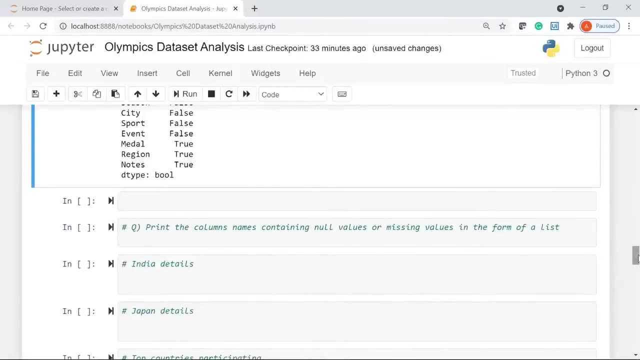 medal region and notes columns that have missing values. so hence it has given us: true. the rest of the columns do not have any nan or missing values, hence they are false. alright, let me scroll down now. let's see the total number of null values for the above. 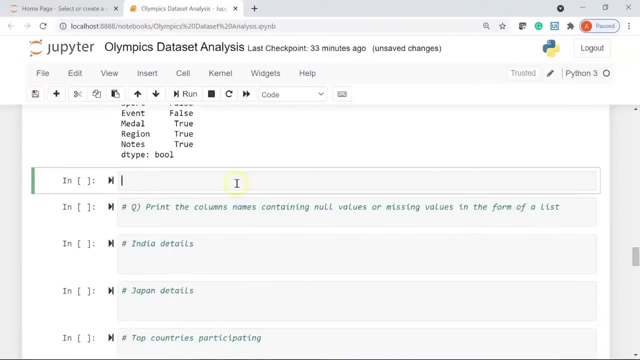 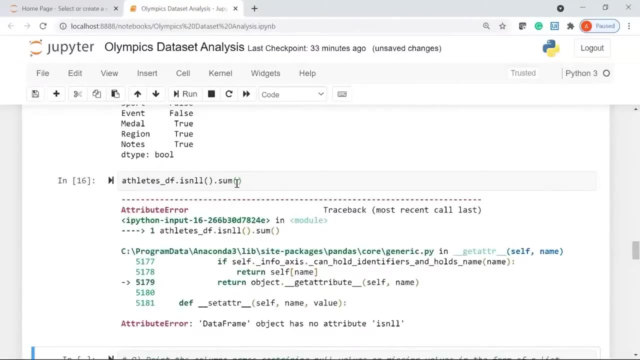 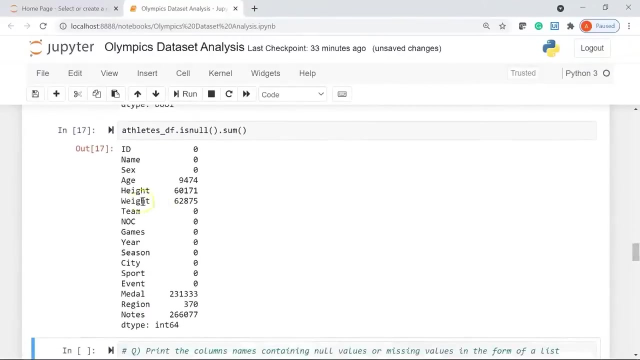 six columns. so i will say athletes. underscore df, dot. i will use the function is null and again i will use the sum function. ok, this should be is null. if i run it, you can see it here. so our age column has 9474 rows where we have. 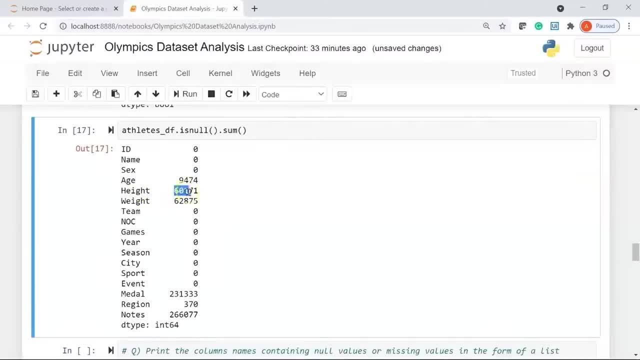 null values. then we have some null values for the height column as well for the weight column. so these are the total number of rows where we don't have any information regarding age, height, weight or region notes. this medal is self explanatory because a lot of the athletes who participate 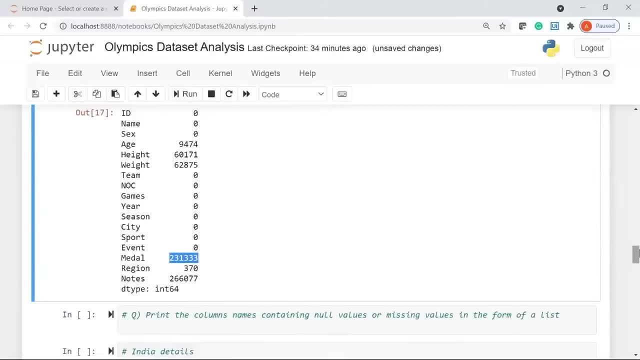 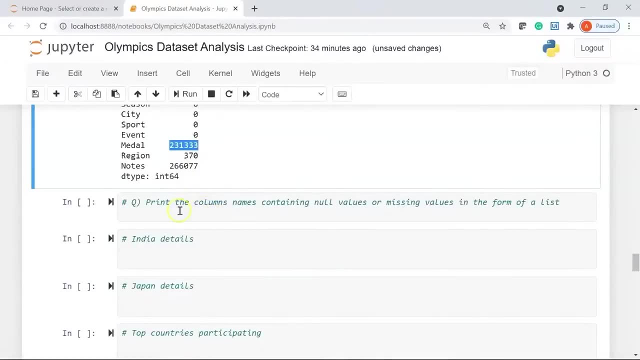 in olympics don't win any medals, so for them the value is any. now, before i move ahead, i have a question for you people. so the question is: i want you to print the column names containing null values or missing values in the form of a list. so 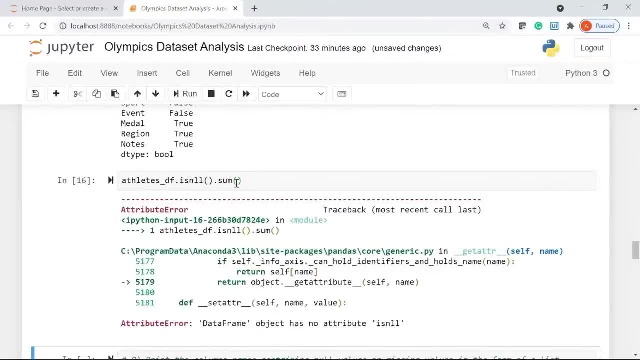 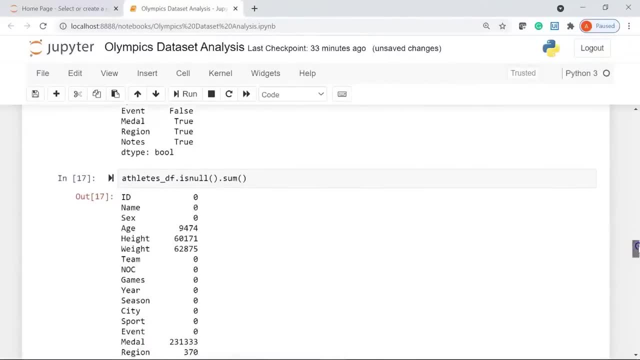 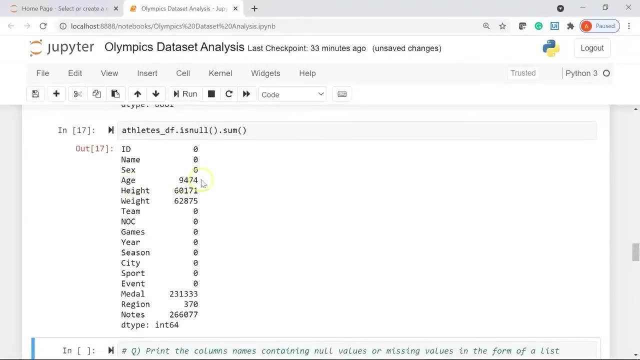 is null and again i will use the sum function. ok, this should be- is null. if i run it, you can see it here. so our age column has 2474 rows where we have null values. then we have some null values for the height column as well for the weight column. 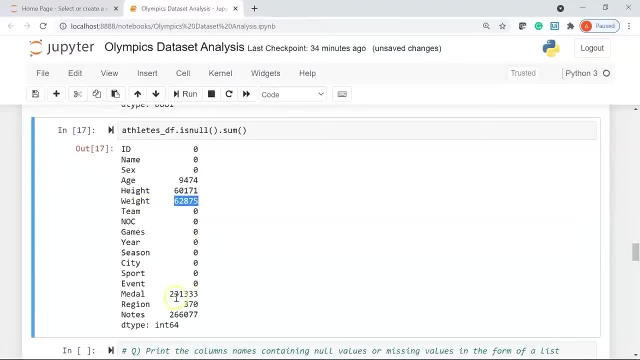 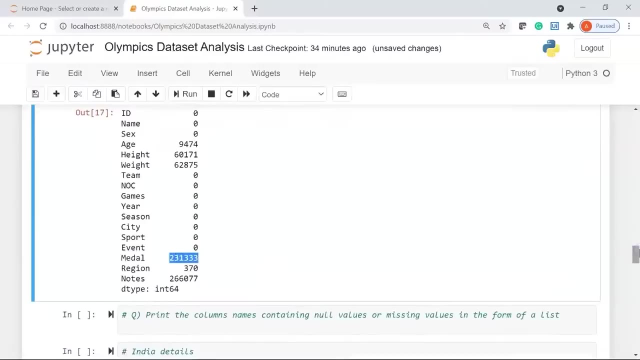 so these are the total number of rows where we don't have any information regarding age, height, weight or region notes. this medal is self explanatory because a lot of the athletes who participate in olympics don't win any medals, so for them the value is any. now before. 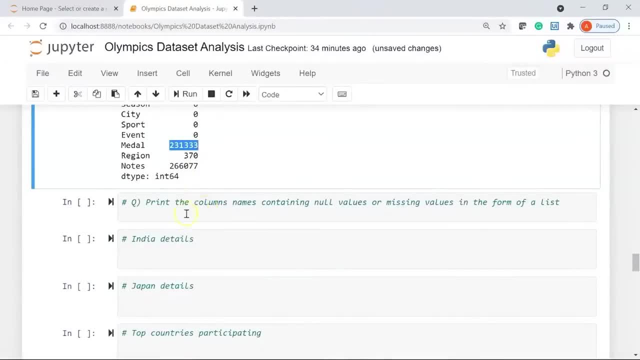 i move ahead. i have a question for you people. so the question is: i want you to print the column names containing null values or missing values in the form of a list. so please answer this question and put it in the comment section of the video. we would be happy. 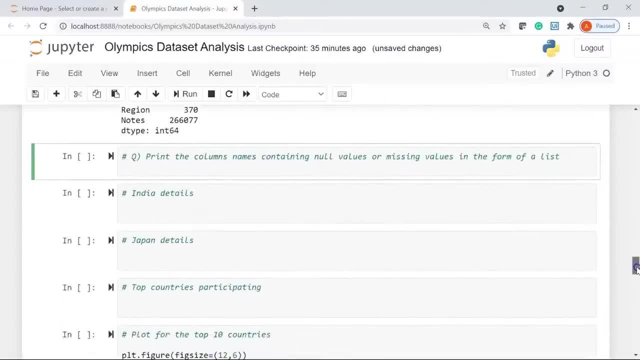 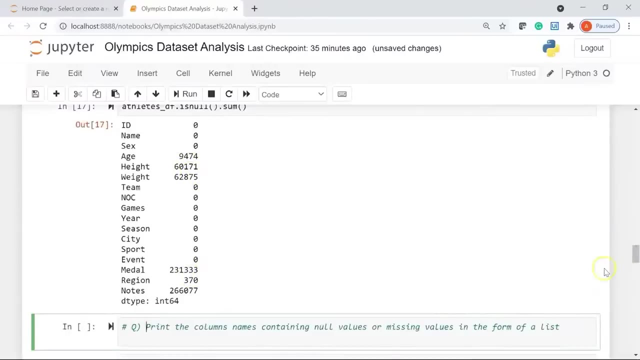 to know your approach. so the question. i will repeat it again: i want you people to print the column names containing null values or missing values in the form of a list. so basically, on the top we saw there were six columns that had null values. i want you to. 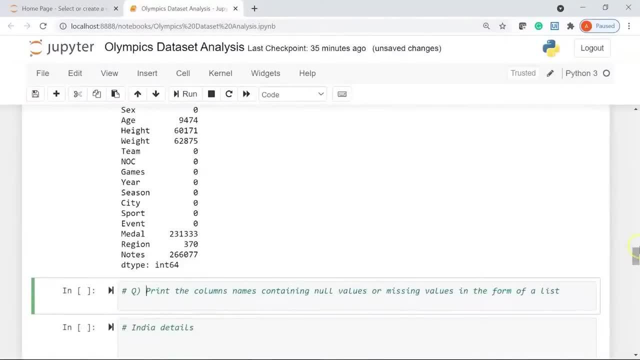 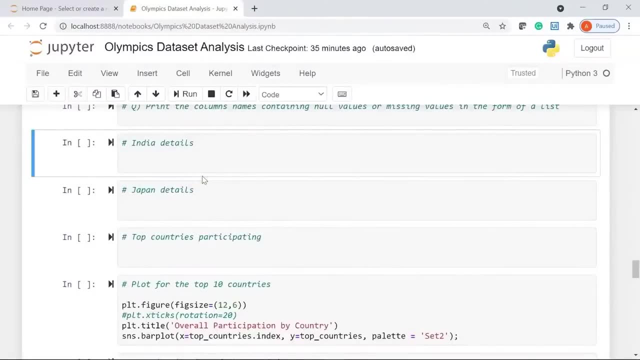 print these six columns in the form of a list. alright, now moving ahead. now let's see the data for specific countries. let's say you want to see the athletes who have participated in the olympic games from the beginning for india. for that you can filter your result. 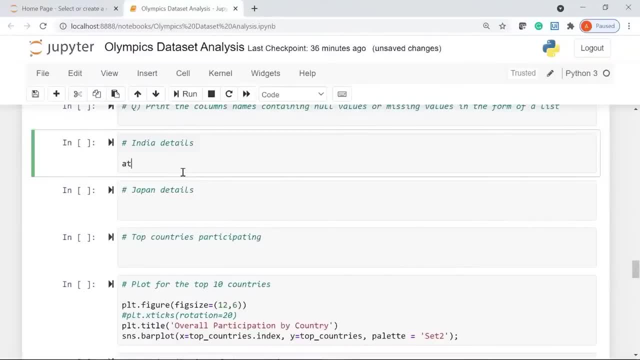 using a function called query. so let me show you how to do it. i will say: athletes, underscore df, dot will use the query function and then i will say: team, which is my column name, should be equal to, equal to, and the value i will give is india. 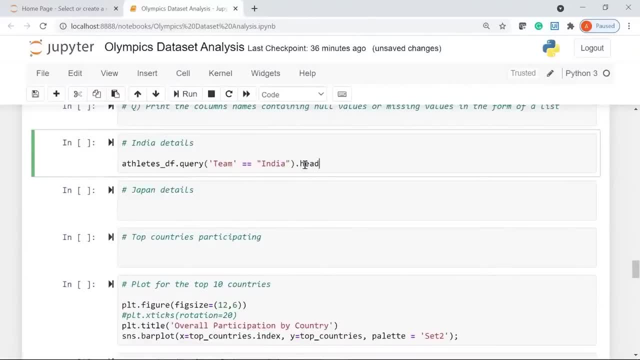 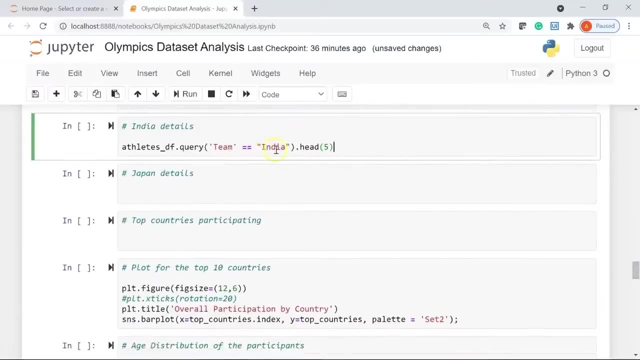 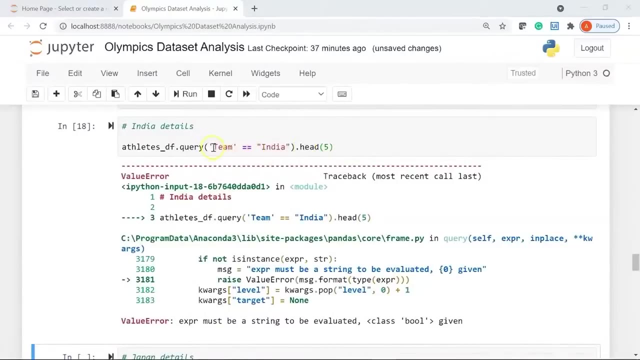 now let's display the first five rows of information, or the details for the athletes who are from india. if i run this, okay, there is some error here. okay, so we need to make sure this entire expression, or the condition, should be within single quote. i will just: 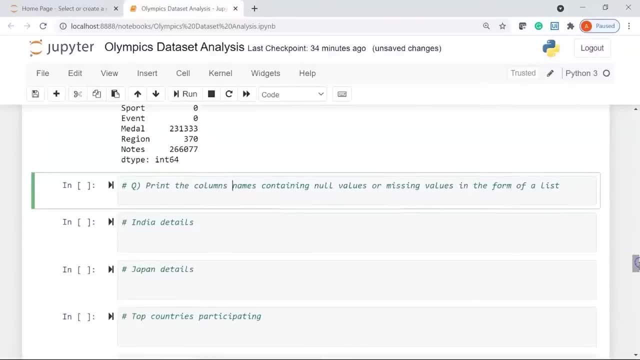 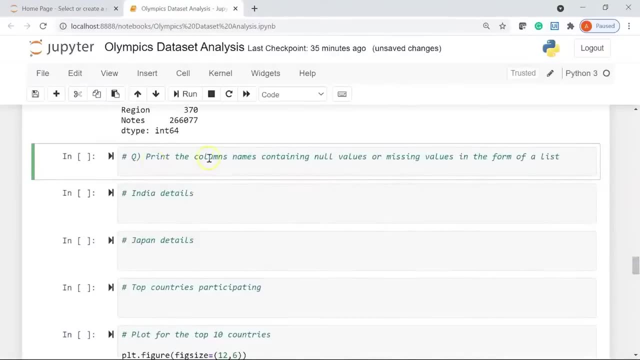 please answer this question and put it in the comment section of the video. we would be happy to know your approach. so the question. i will repeat it again: i want you people to print the column names containing null values or missing values in the form of a list. so basically, 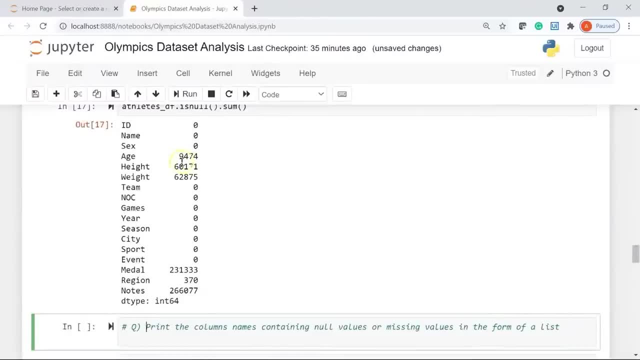 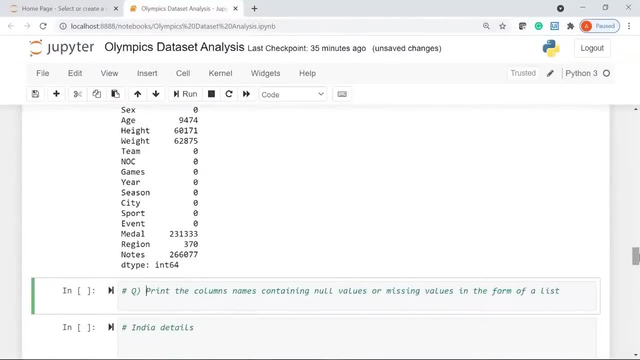 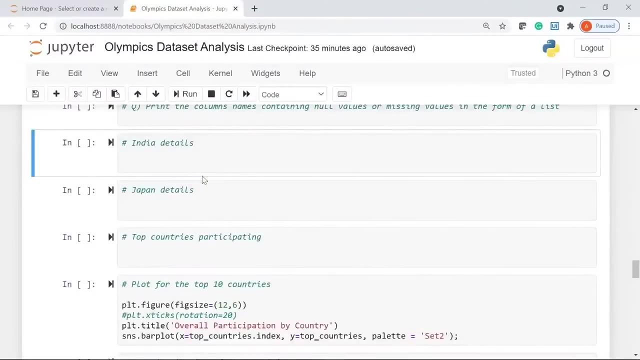 on the top, we saw there were six columns that had null values. i want you to print these six columns in the form of a list. alright, now moving ahead, now let's see the data for specific countries. let's say you want to see the athletes who have participated in the. 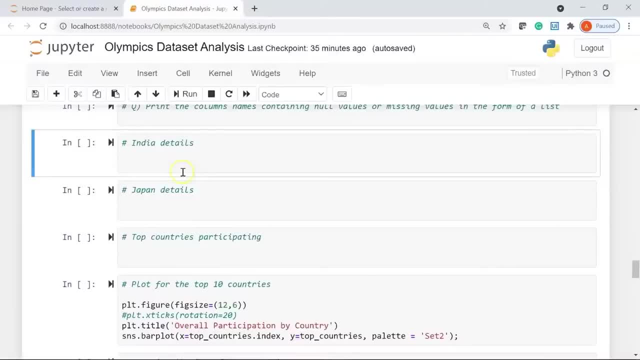 olympic games from the beginning for india. for that you can filter your result using a function called query. so let me show you how to do it. i will say athletes- underscore df, dot, will use the query function and then i will say team, which is my column name should. 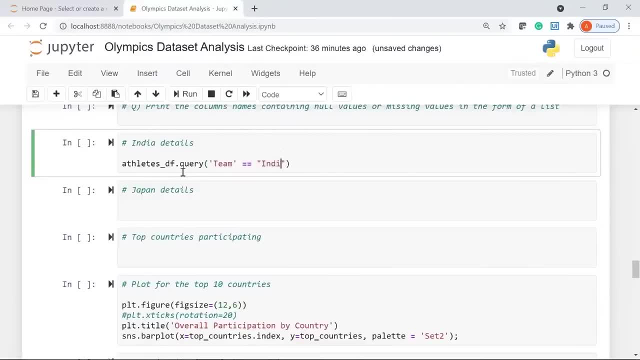 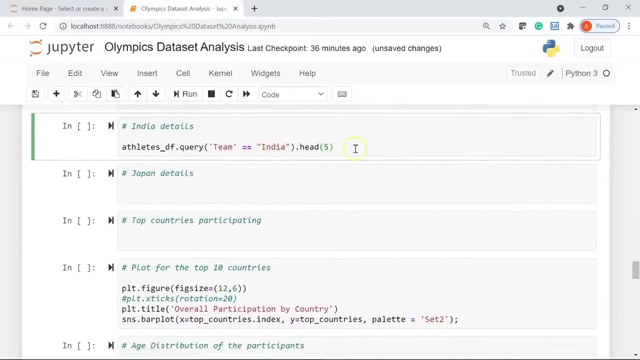 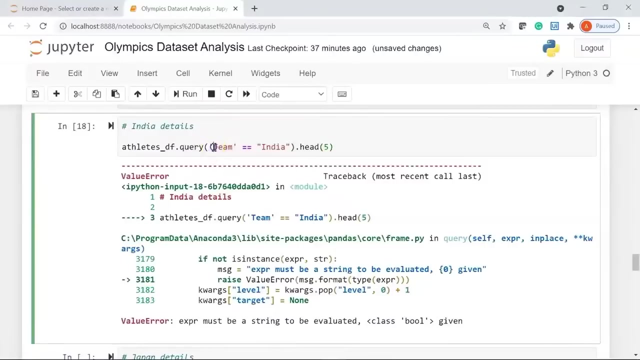 be equal to, equal to, and the value i will give is india. now let's display the first five rows of information, or the details for the athletes who are from india. if i run this, okay, there is some error here, okay, so we need to make sure this entire expression. 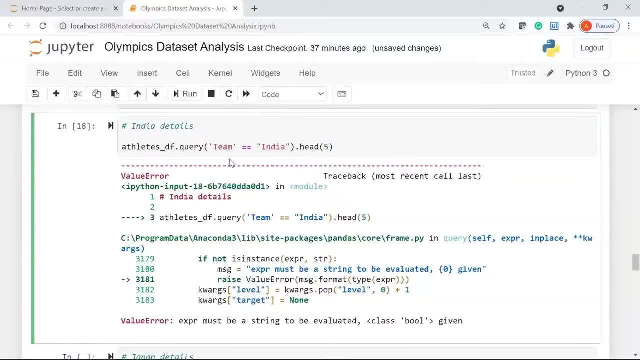 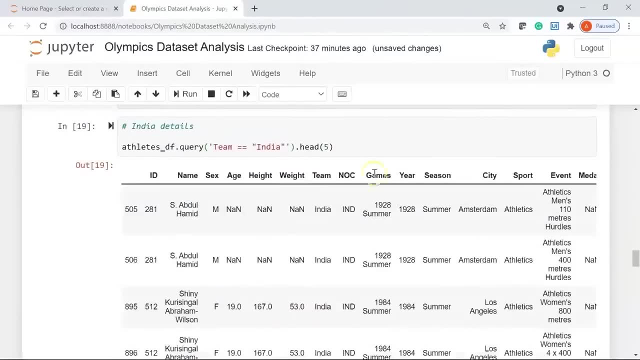 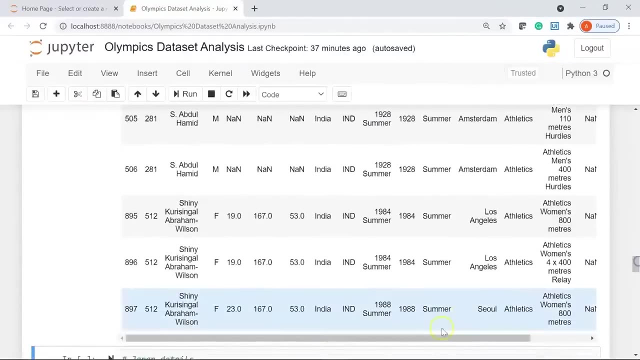 or the condition should be within single quote. i will just delete this single quote from here and we will add it in the end. now let's run it. there you go. so here you can see we have the top five rows of the athletes who are from india. you 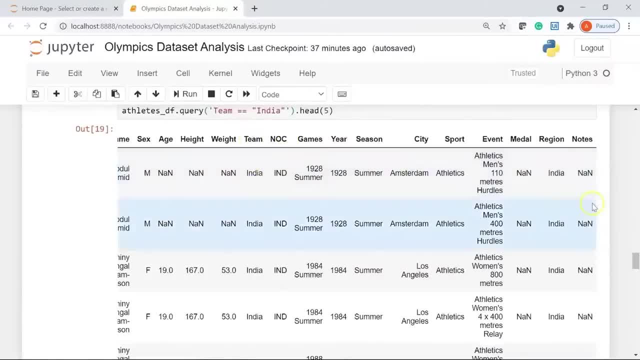 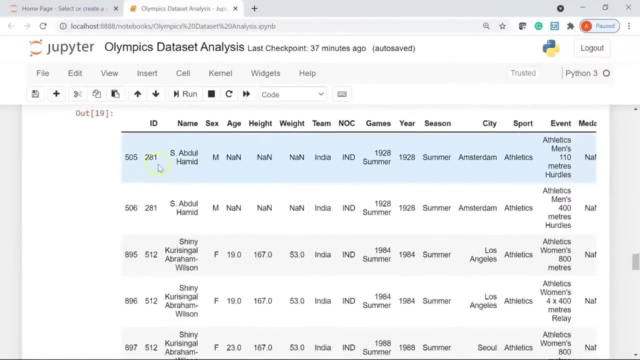 can see here, the region is india, you can see the noc is india, the team is india. and let me go to the left. you can see the name of the athlete, the sex age. so for age you have some missing values. you have the weight, team, year and everything. 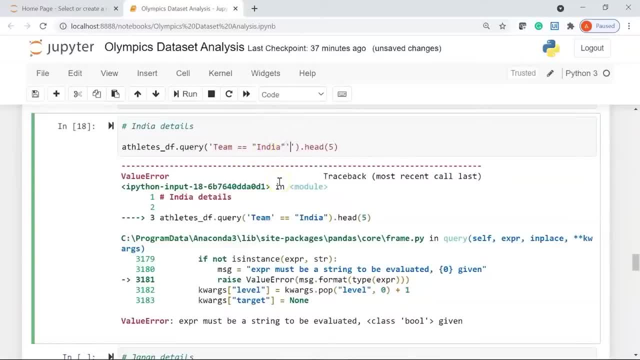 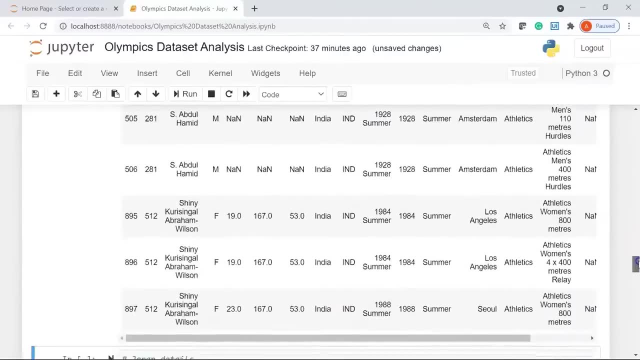 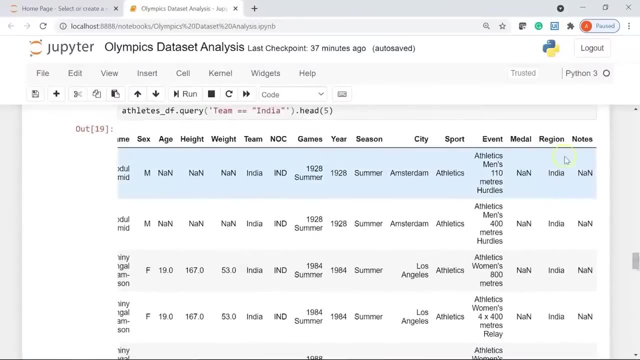 delete this single quote from here and we will add it in the end. now, let's run it. there you go. so here you can see, we have the top five rows of the athletes who are from india. you can see, here the region is india, you can see. 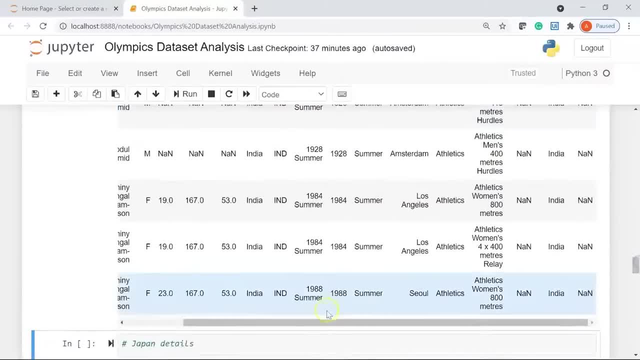 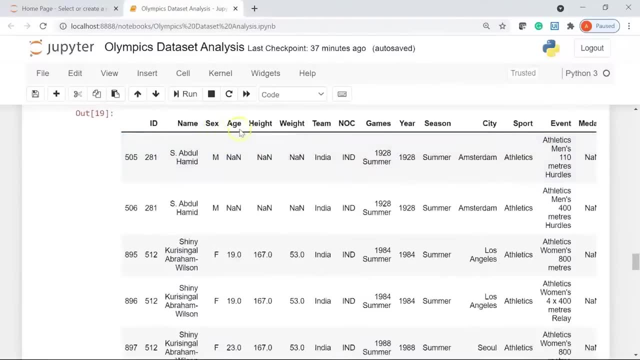 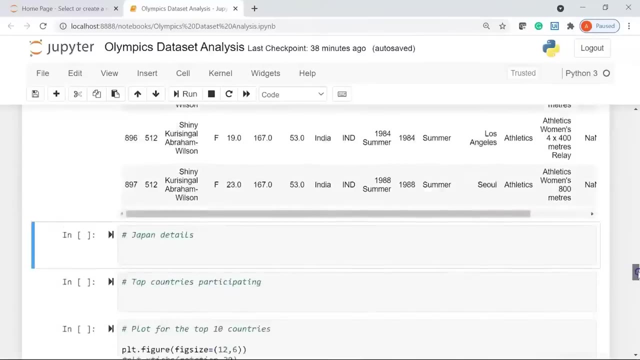 the noc is india, the team is india, and let me go to the left. you can see the name of the athlete, the sex age. so for age, you have some missing values. you have the weight team year and everything all right. similarly, you can also check for japan. 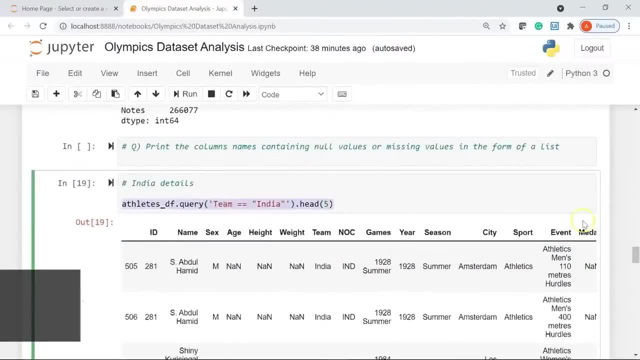 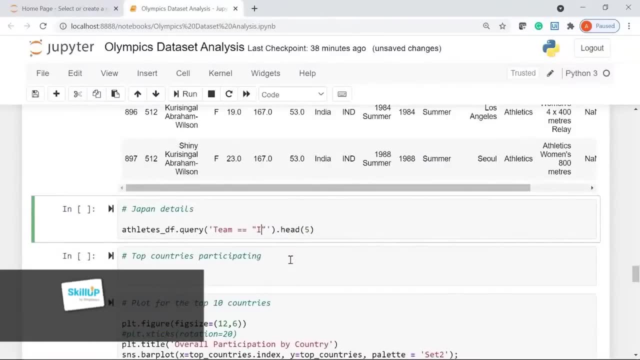 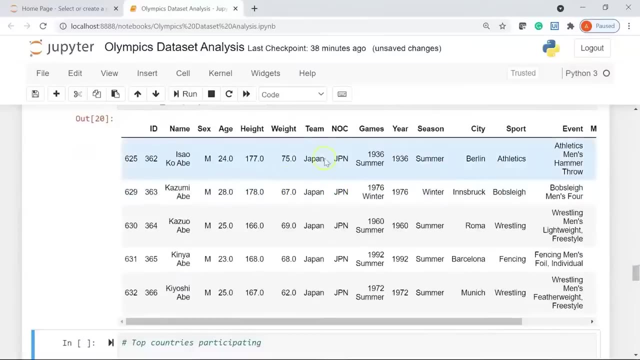 let me just copy the above code, i will paste it here and instead of india i will say japan. i will run it there you go. so if you see, here you can see all the details are for the athletes who are from japan. all right now, moving ahead. now i will. 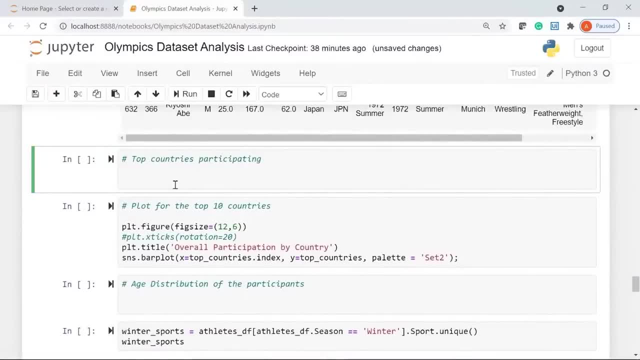 want to know the top 10 countries who have participated since the inception of olympics in 1896. so for that i will create a variable called top underscore. 10 underscore countries i will say equal to- i will use my data frame, that is athletes underscore. 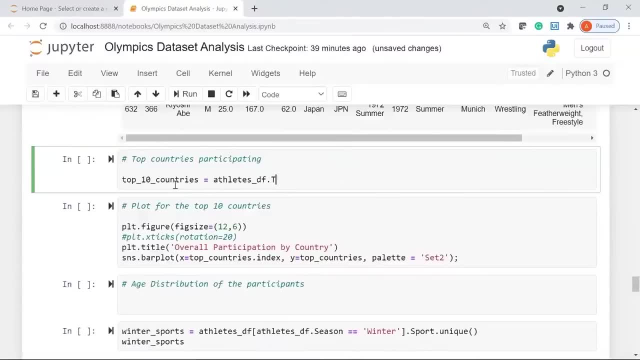 tf, i will say dot team, then i will use the function value underscore counts. i am going to sort my count in ascending order. just mark the way in which i am writing the functions. any error in terms of syntax of the flow will throw you an error. i want 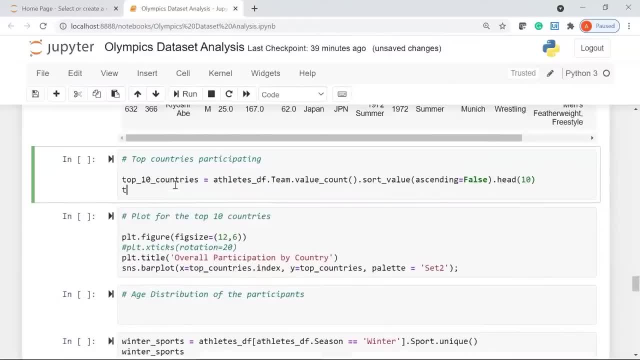 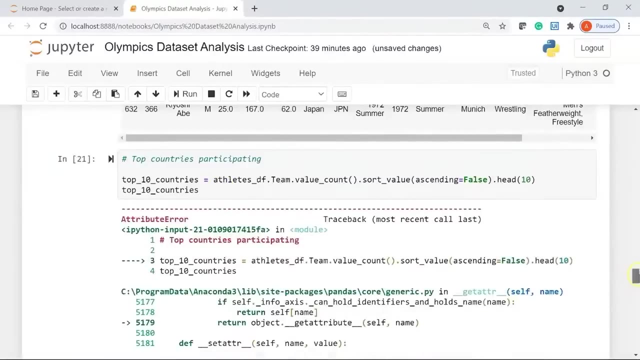 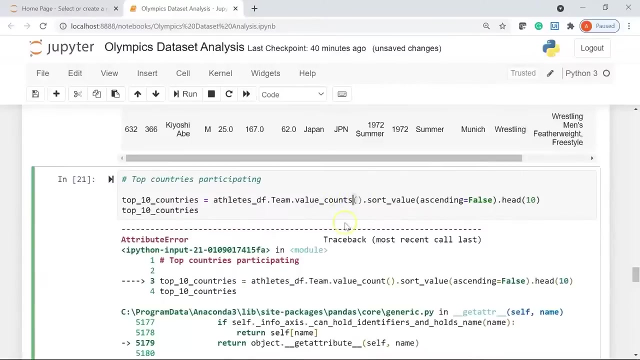 to display the top 10 countries. now let's go ahead and print it. i will say: top underscore 10 underscore countries. all right, let me run it okay. it has given us an error. let's debug it, okay. so this should be value counts and not count. let's run it again. 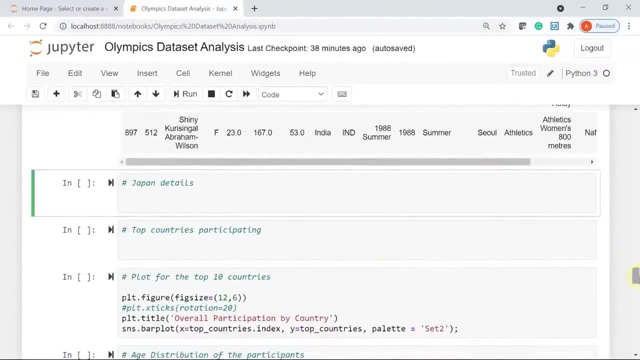 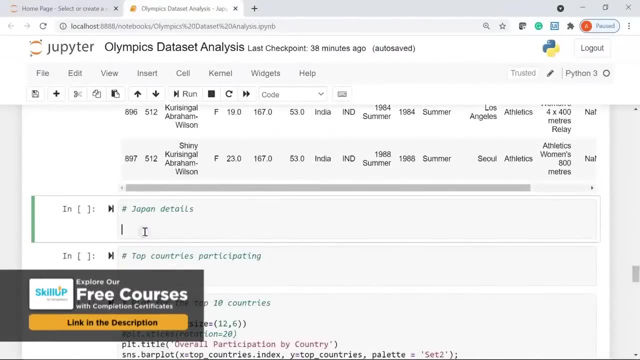 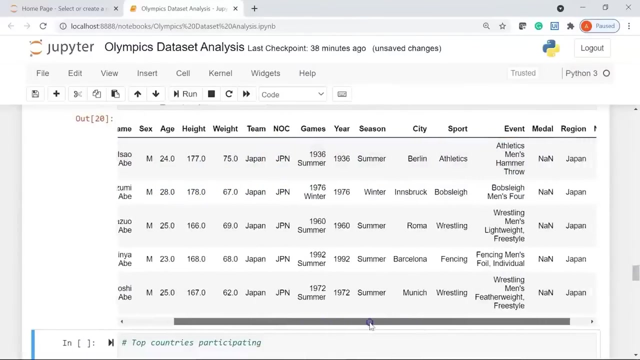 alright. similarly, you can also check for japan. let me just copy the above code, i will paste it here and instead of india i will say japan. i will run it there you go. so if you see, here you can see all the details are for the athletes who are from japan. 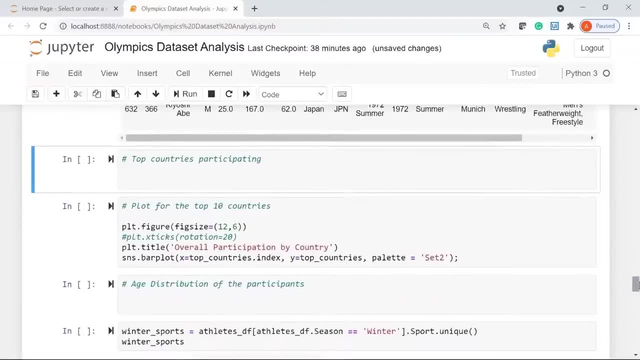 alright, now moving ahead. now i want to know the top ten countries who have participated since the inception of olympics in 1996. so for that i will create a variable called top underscore. ten underscore countries i will say equal to. i will use my data frame, that is. 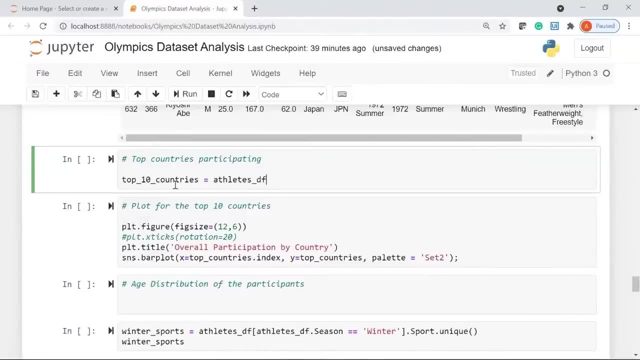 athletes. underscore tf. i will say dot team, then i will use the function value. underscore counts. i am going to sort my count in ascending order. just mark the way in which i am writing the functions. any error in terms of syntax of the flow will throw you an error. 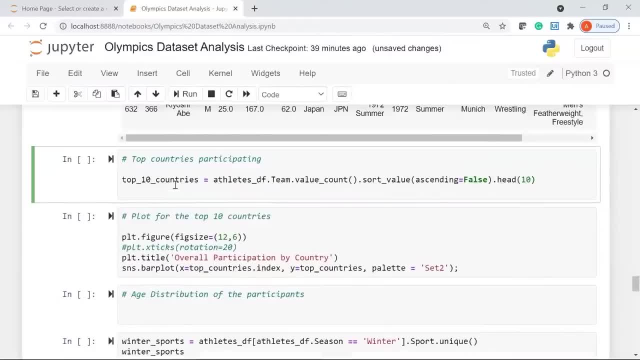 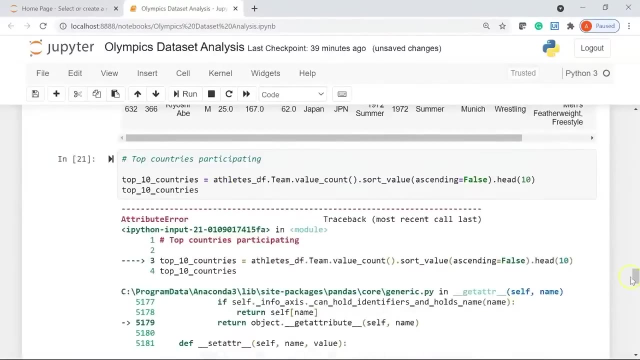 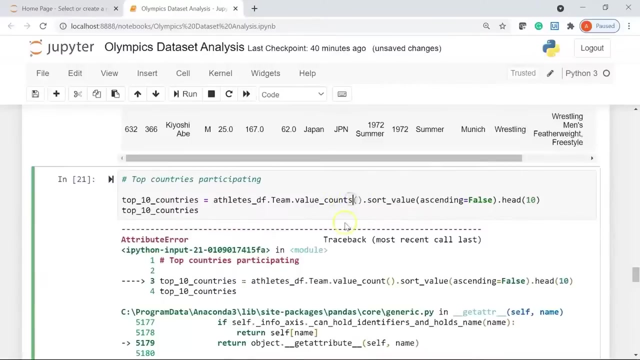 i want to display the top ten countries. now. let's go ahead and print it. i will say: top underscore, ten underscore countries. alright, let me run it. ok, it has given us an error. let's debug it. ok. so this should be value counts and not count. let's run it again. 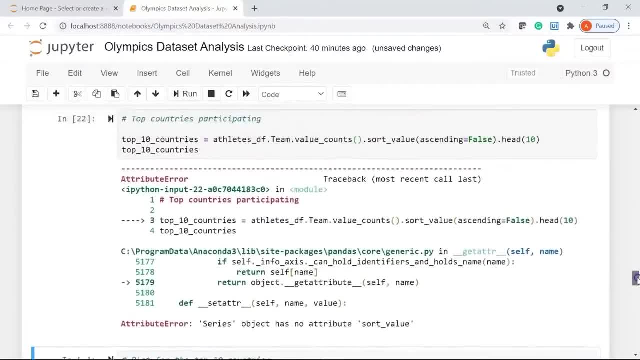 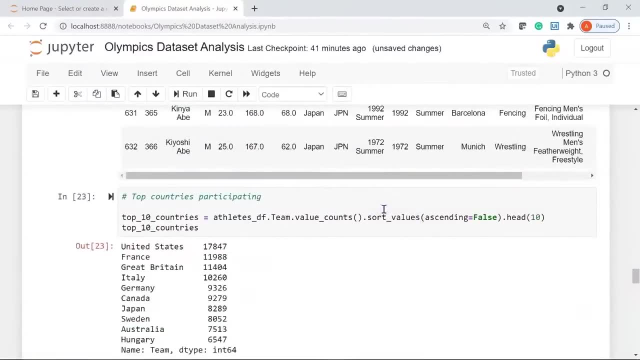 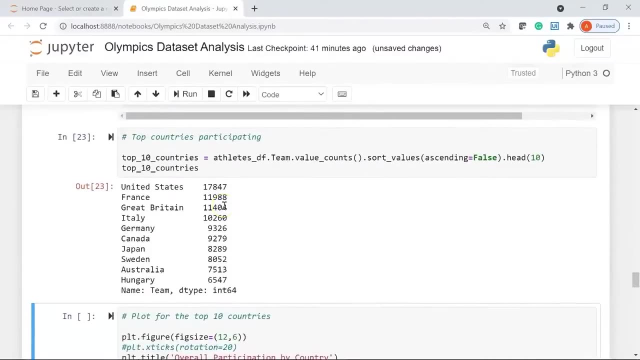 another error. ok, so this should be short underscore values and not value. let's run it again. there you go. so here you can see the top ten countries participating in olympics since 1896. you have united states, then we have france, so these are the. 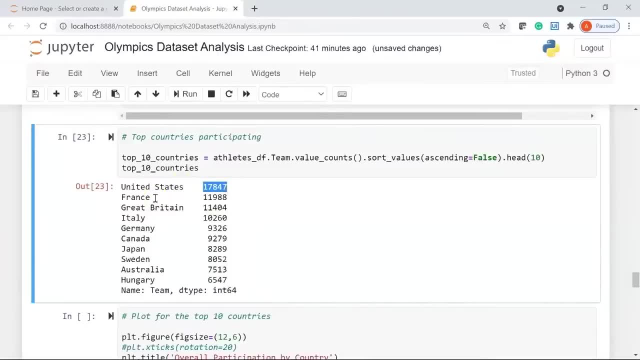 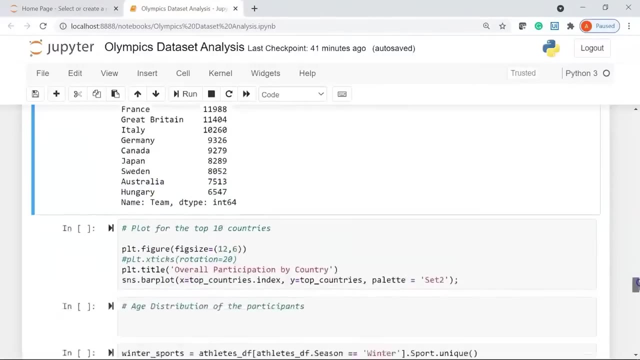 number of participants who have taken part since 1896. so the most number of participants have come from us. then we have france, great britain, italy, germany, canada, japan, sweden. we also have australia and hungary. i will scroll down now we are going to. 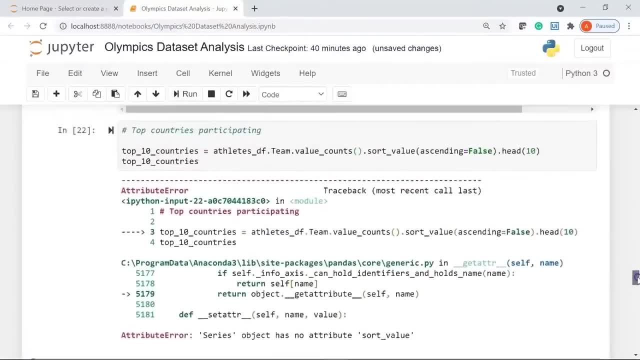 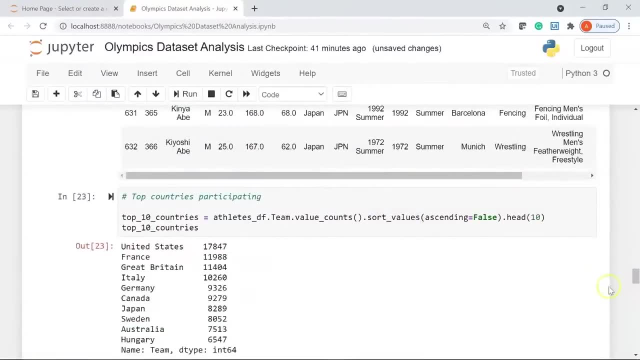 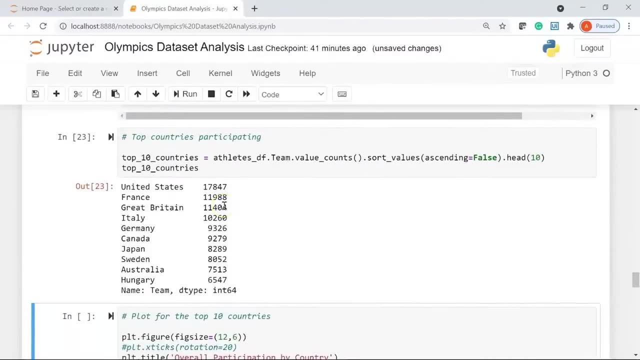 another error. okay, so this should be short underscore values and not value. let's run it again. there you go. so here you can see the top 10 countries participating in olympics since 1896. you have united states, then we have france, so these are the number of 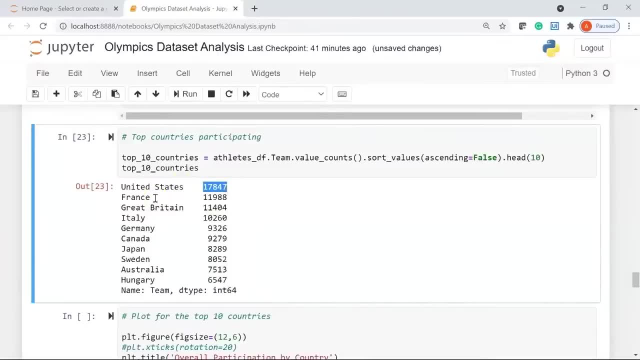 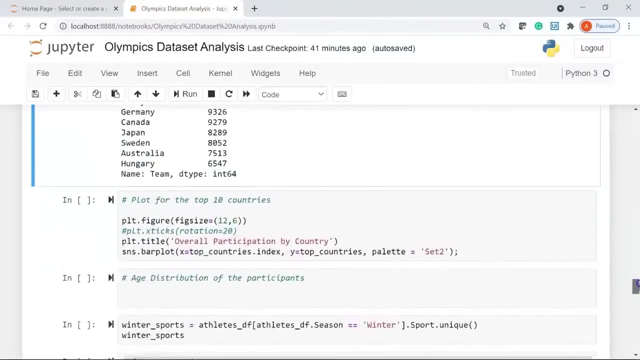 participants who have taken part since 1896, so the most number of participants have come from us. then we have france, great britain, italy, germany, canada, japan, sweden. we also have australia and hungary. i will scroll down now. we are going to convert this table. 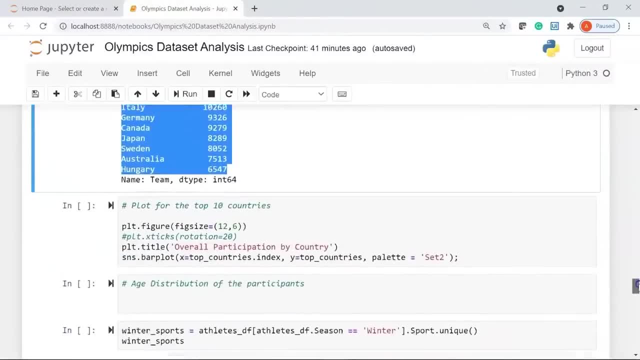 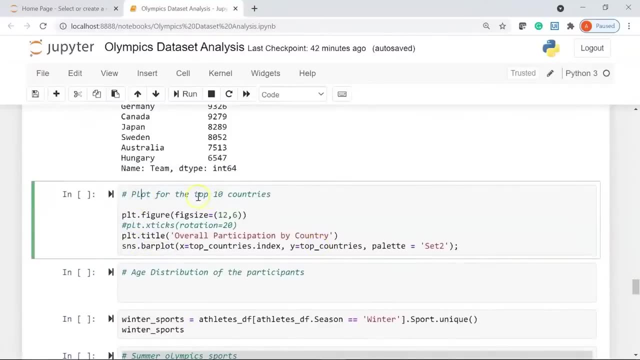 that we got, or the output that we got in the form of a graph. so i am trying to create a bar plot to plot the top 10 countries who have participated in olympics. so here i am using the figure function to give the figure size. so these are the dimensions. 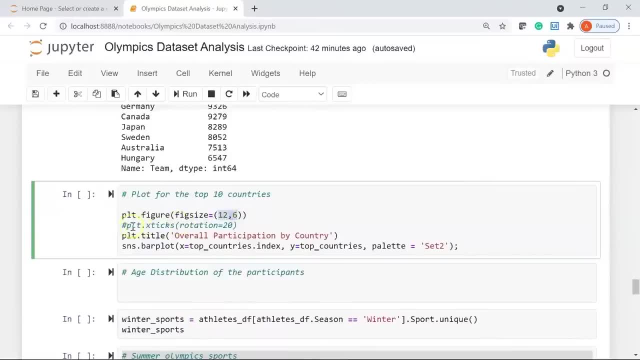 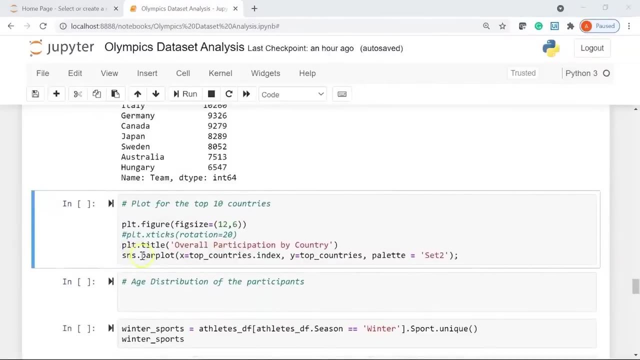 12 comma 6. now i will tell you what this plt x text means. just wait for a while. i have given a title to my plot saying overall participation by country, and then, using the seaborn library and the bar plot function, i am plotting the x and the. 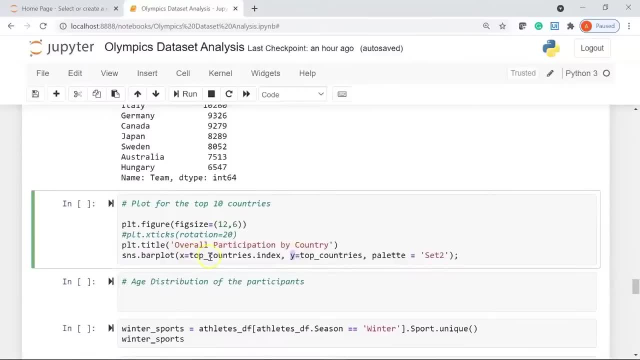 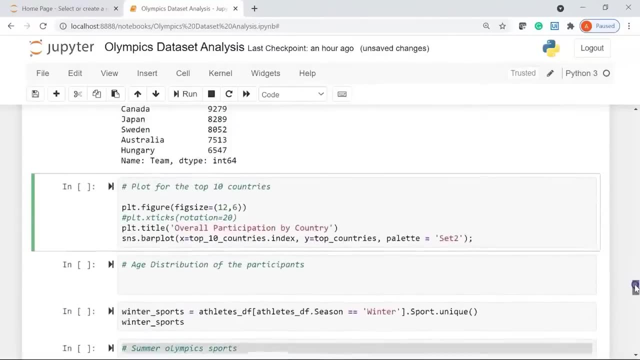 y axis, so my x axis has top. i should make this top 10 countries, because above we used top underscore- 10 underscore countries. similarly for y axis, i will make it top underscore- 10 underscore countries. and then i am using a color palette called set 2. 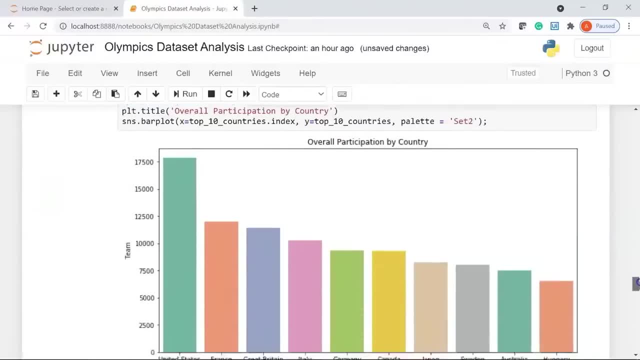 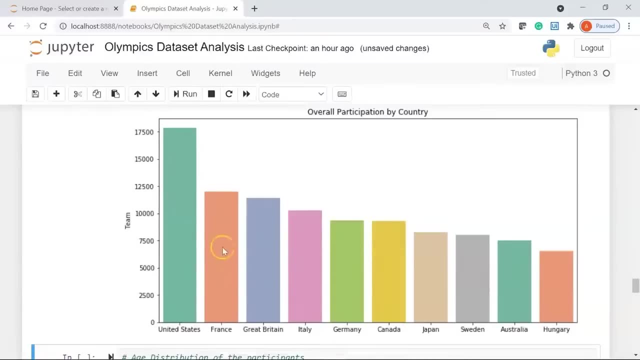 let's run it. there you go. so if i scroll down you can see here we have a nice bar plot. this is a vertical bar plot and here you can see the bars which represent the different country names. first we have united states, which has the highest participation. 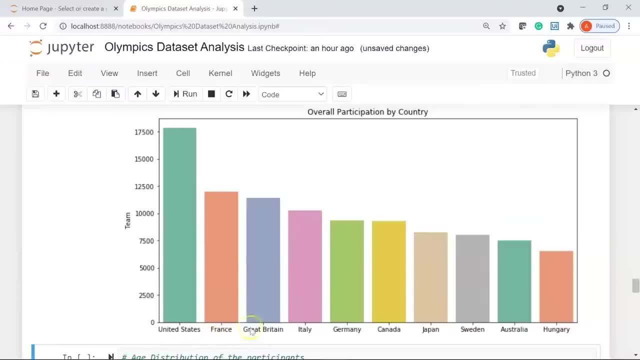 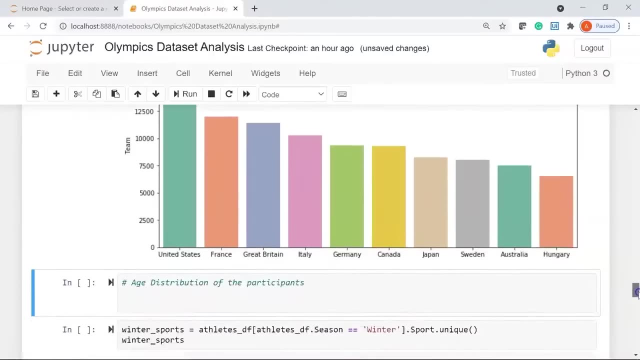 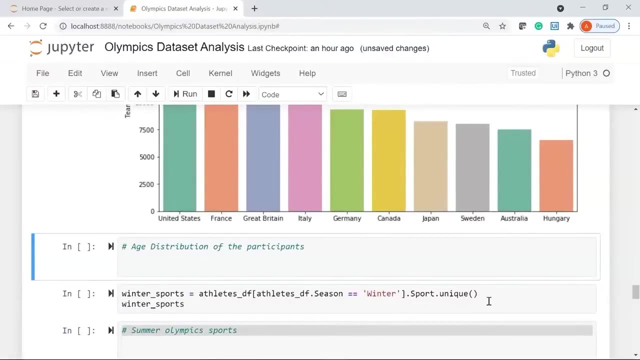 since the beginning of the olympics. then we have france, great britain, italy, germany, canada, and we have the rest of the countries- cool now moving ahead. the next visualization we are going to see is the age distribution of the athletes. so for this we are going to 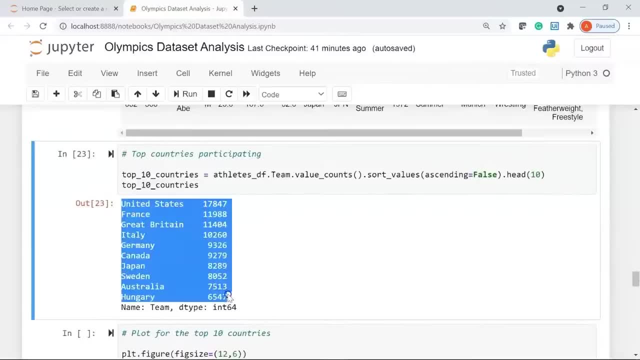 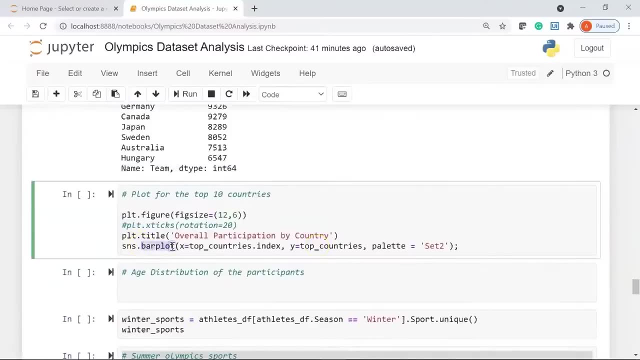 convert this table that we got or the output that we got in the form of a graph. so i am trying to create a bar plot to plot the top ten countries who have participated in olympics. so here i am using the figure function to give the 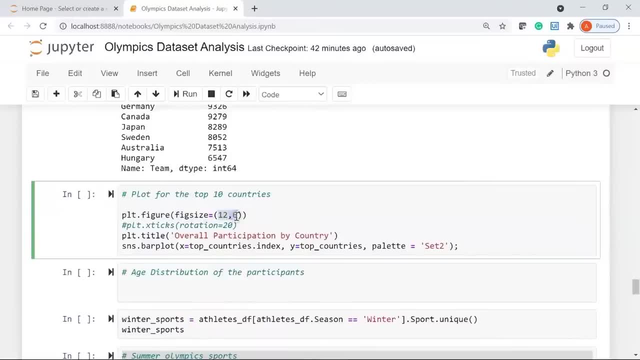 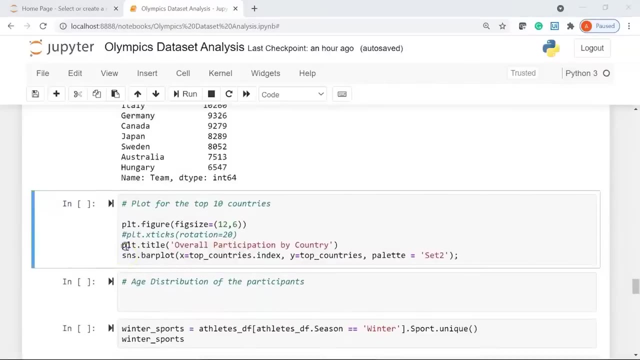 figure size. so these are the dimensions. 12 comma 6. now i will tell you what this plt x tics means. just wait for a while. i have given a title to my plot saying overall participation by country and then, using the seaborn library and the bar plot function. 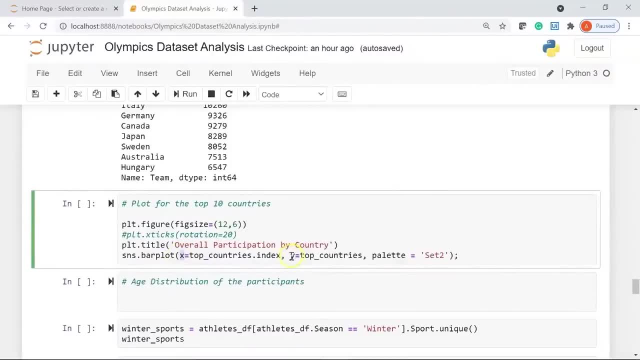 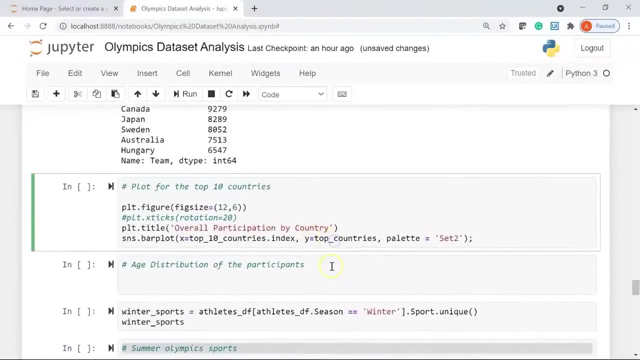 i am plotting the x and the y axis, so my x axis has top. i should make this top 10 countries, because above we used top underscore- 10 underscore countries. similarly for y axis, i will make it top underscore- 10 underscore countries. and then i am using a color palette called. 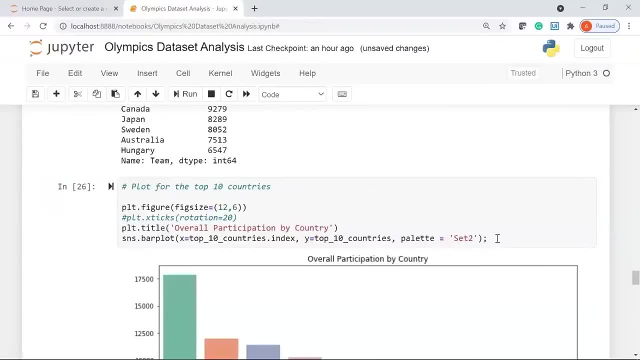 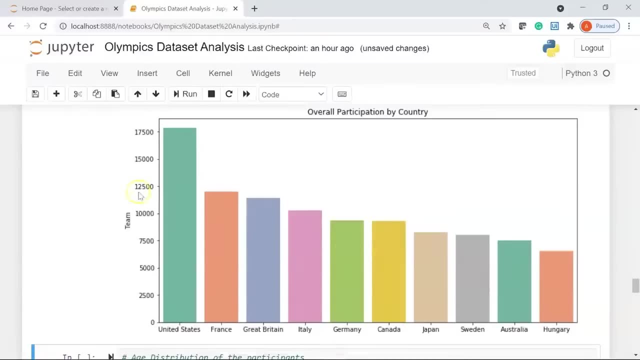 set 2. let's run it there you go. so if i scroll down you can see here we have a nice bar plot. this is a vertical bar plot and here you can see the bars which represent the different country names. first we have united states, which has the highest. 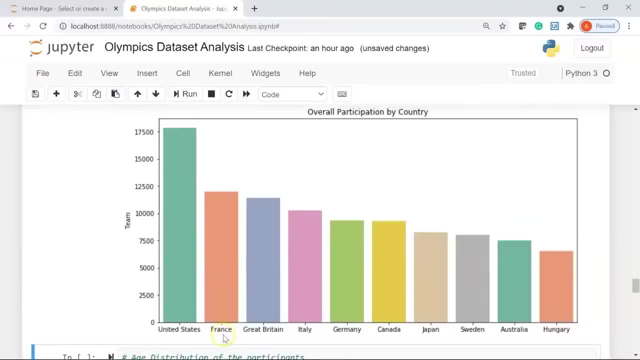 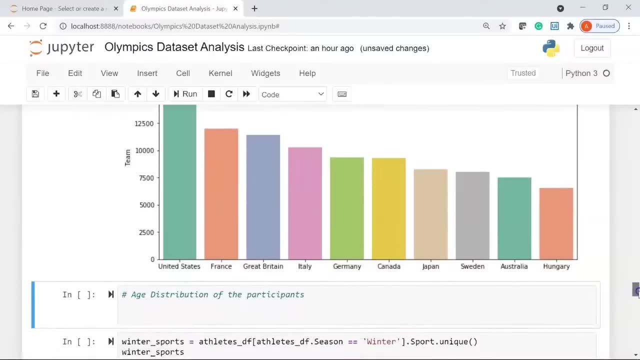 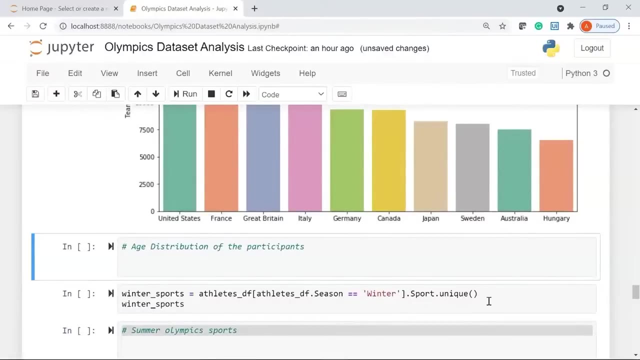 participation since the beginning of the olympics. then we have france, great britain, italy, germany, canada, and we have the rest of the countries- cool now moving ahead. the next visualization we are going to see is the age distribution of the athletes. so for this we are going. 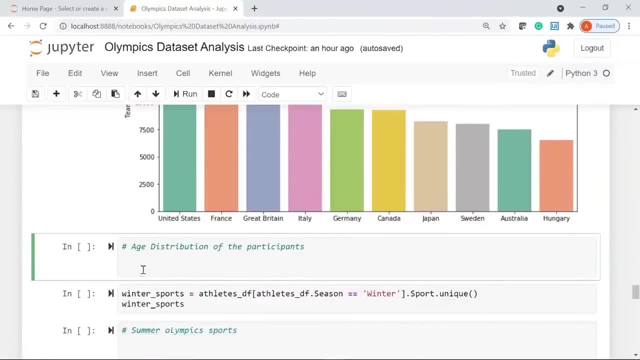 to create a histogram. i will be using the matplotlib library specifically for this visualization. so i will say: plt, dot figure will give the figure size using the argument fig size equal to, and this will be a tuple. actually, my size is going to be 12 comma 6. 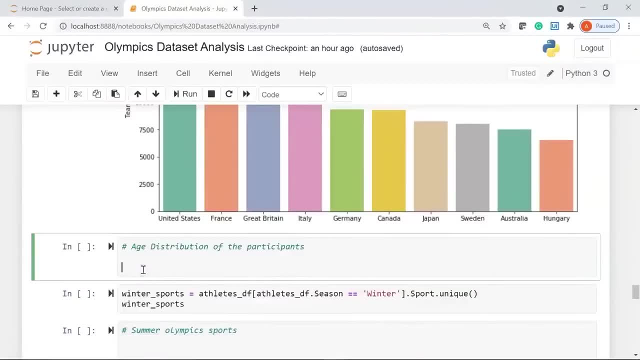 create a histogram. i will be using the matplotlib library specifically for this visualization. so i will say: plt, dot figure will give the figure size using the argument fig size equal to, and this will be a tuple. actually, my size is going to be 12 comma 6. 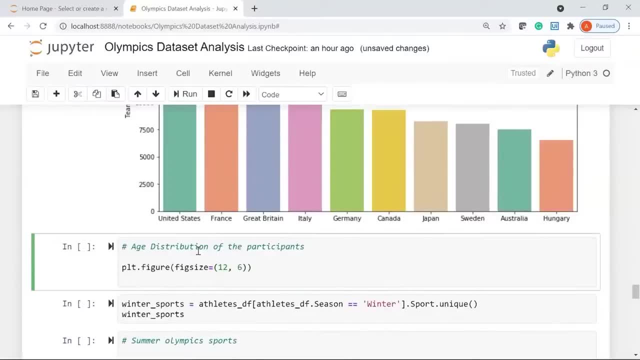 i will say plt dot title. now you can give any title that you want. i will say plt dot- age- distribution of the athletes. then we will also give the x labels. i will say plt dot x label. this will have age. then we will say plt dot y label. 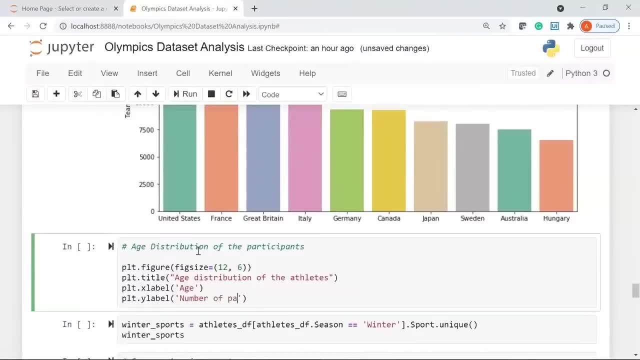 and this will have number of participants. next, i am going to use the hist function, so i will say plt, dot, hist and i will pass in my data frame that is athletes, underscore df, dot age, which is my column name comma. i am going to pass in the 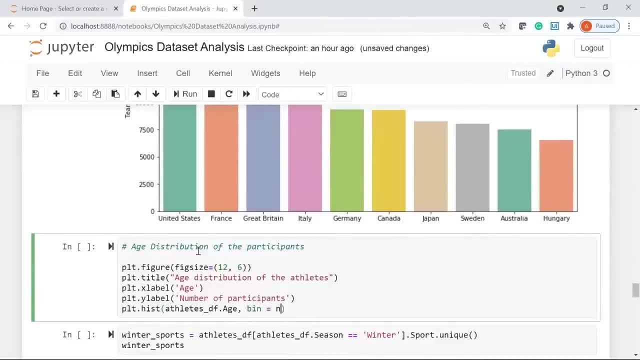 bins. for that i am going to use the np dot arange function. so mp is for numpy and inside this i will say 10 comma 80, comma 2. so my bins will start from the value 10 and go until 80 with a size of 2. 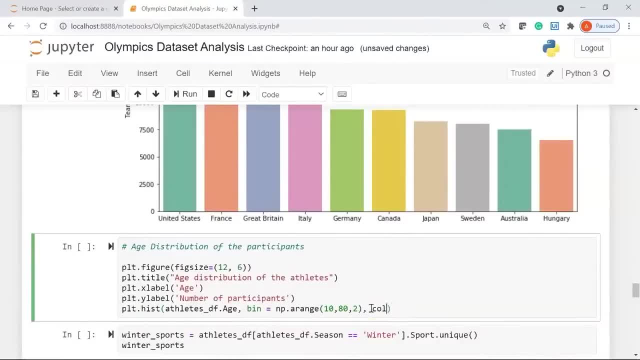 comma. i will give another parameter that is going to specify the color of the bins. i want my color to be orange and then i will use the edge color to separate the bins. i will say edge color. this is the parameter or the argument name and the color. 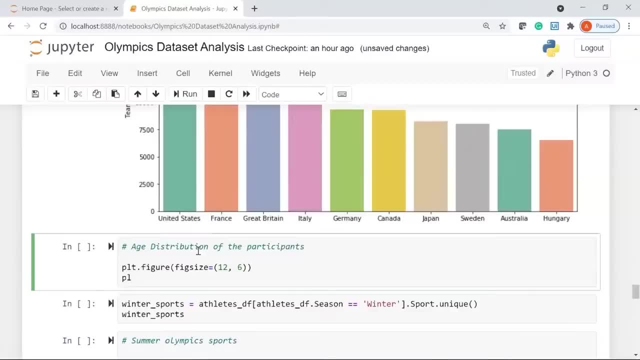 i will say plt dot title. now you can give any title that you want. i will say age: distribution of the athletes. then we'll also give the x labels. i'll say plt dot x label. this will have age. then we'll say plt dot y label and this will have. 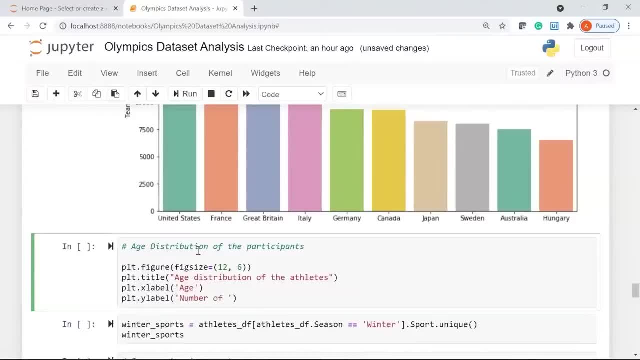 the label as number of participants and next i'm going to use the hist function, so i'll say plt, dot, hist and i'll pass in my data frame. that is athletes underscore: df, dot age, which is my column name comma. i'm going to pass in the bins. 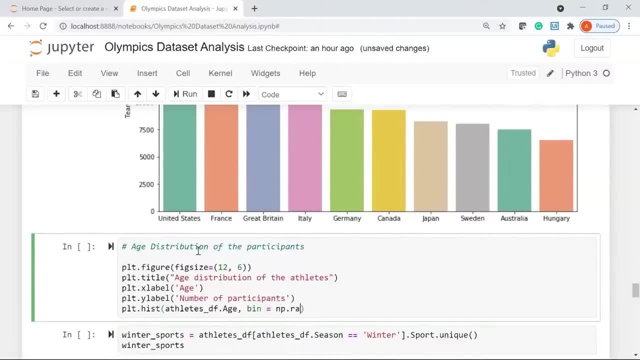 for that i'm going to use the np dot range function. so mp is for numpy and inside this i'll say 10 comma 80, comma 2. so my bins will start from the value 10 and go until 80 with a size of 2. 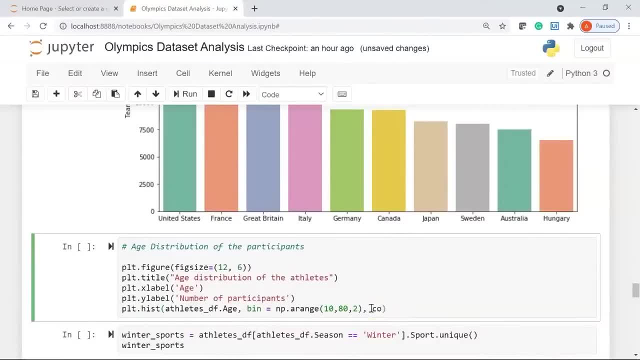 comma. i'll give another parameter that is going to specify the color of the bins. i want my color to be orange and then i'll use the edge color to separate the bins. i'll say edge color. this is the parameter or the argument name, and the color i want is white. 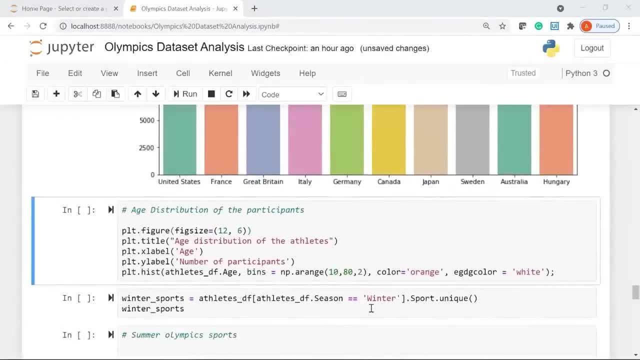 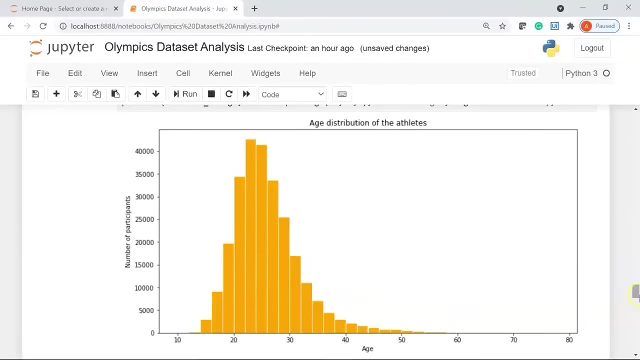 let's give a semicolon here, and this should be edge color. there's a spelling mistake here. now let's run it and we'll see the output. so there you go. so this is a nice histogram that shows the distribution of the age of the athletes. you can see the 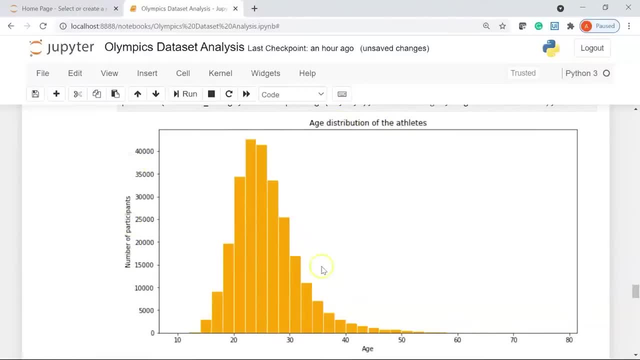 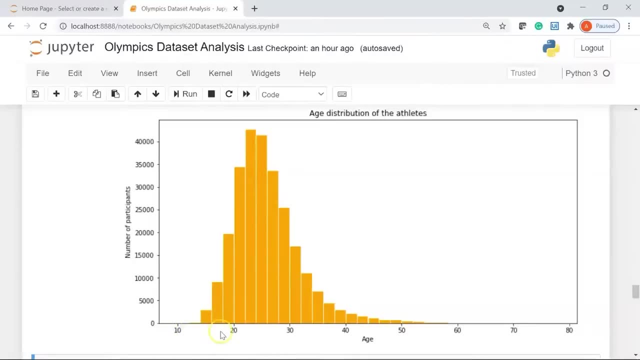 title: age: distribution of the athletes. on the y-axis you have the number of participants. on the x-axis, we have the age values ranging from 10 to 80, with a size of 2, and, if you see this, we have most number of athletes who have a age between: 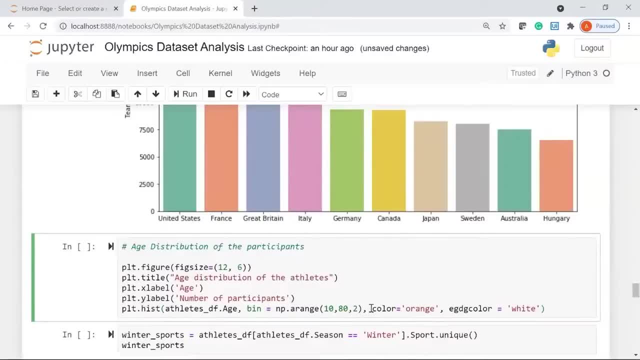 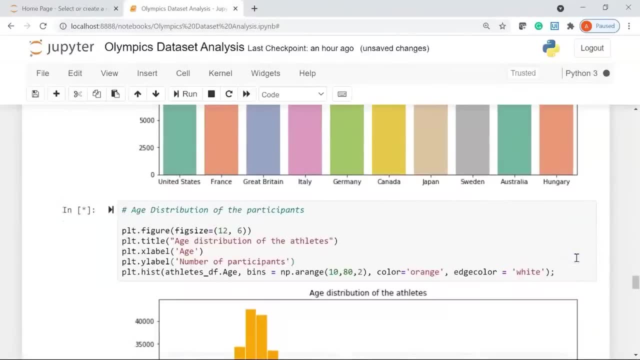 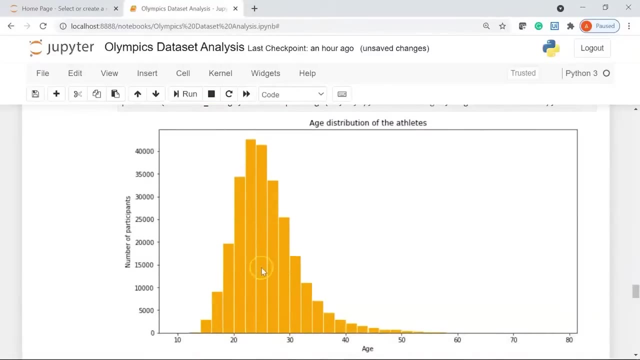 i want is white. let's give a semicolon here, and this should be edge color. there is a spelling mistake here. now let's run it and we will see the output. so there you go. so this is a nice histogram that shows the distribution of the age. 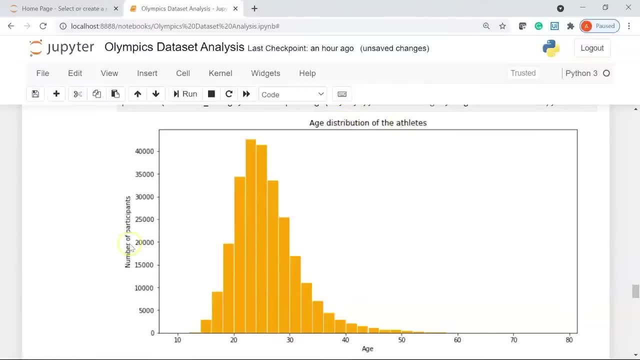 of the athletes. you can see the title: age distribution of the athletes. on the y-axis you have the number of participants. on the x-axis we have the age values ranging from 10 to 80, with a size of 2, and if you see this, we have. most number of athletes who have age between 20 to 30. you can see here: so early 20s, we have maximum number of athletes participating in the olympics. we also have a few athletes who are beyond 40 years of age. you can see here we have 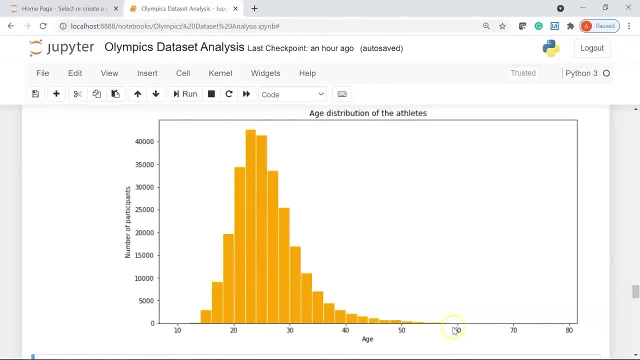 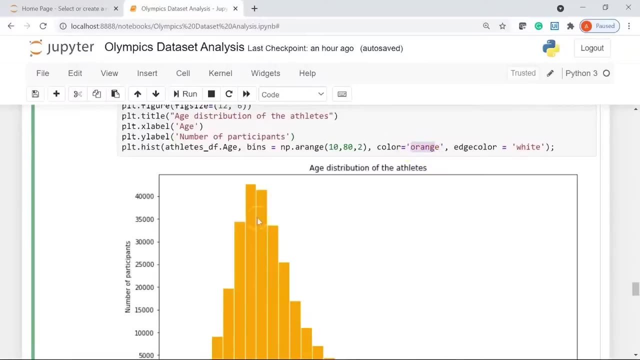 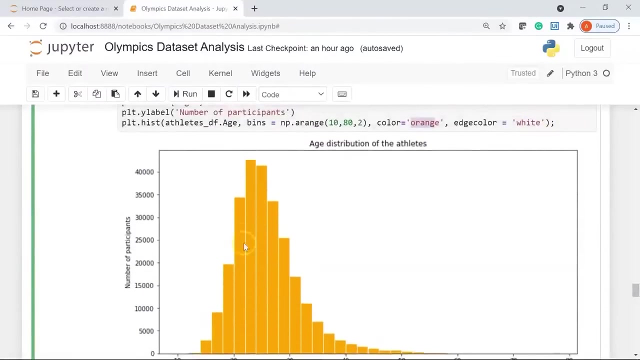 a few athletes even closer to 60 also, and similarly, we have a few athletes who are under 18 years of age. alright, now you can see here the bins. we had taken orange color, so all the bars are represented in orange color and the edge you can see here we have the white color. 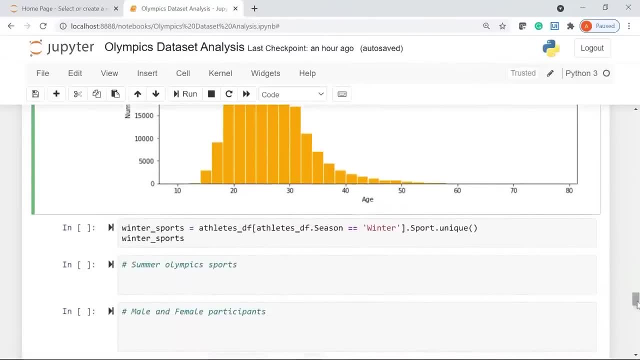 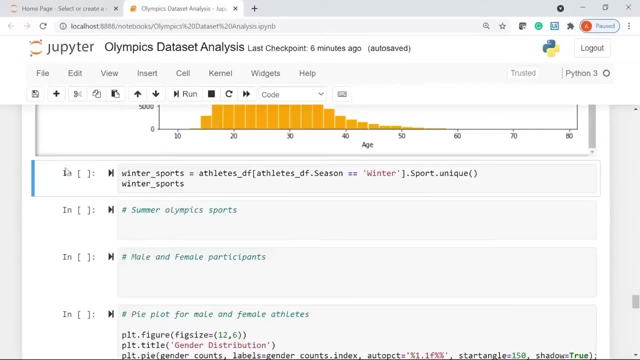 alright, now moving ahead. now, in the initial slides of the video we discussed the summer and winter olympic games. let's look at the different sporting events that are part of the summer and winter olympic games. just to give you a heads up, the winter olympic games are: 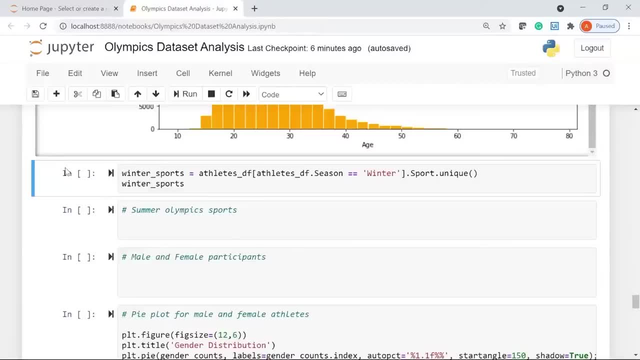 held once every 4 years for sports practiced on snow and ice. so here i have my variable name: winter sports. so i am extracting for season equal to equal to winter and i am going to display only the unique values. now let me run this cell, ok, so you can see here. these are the 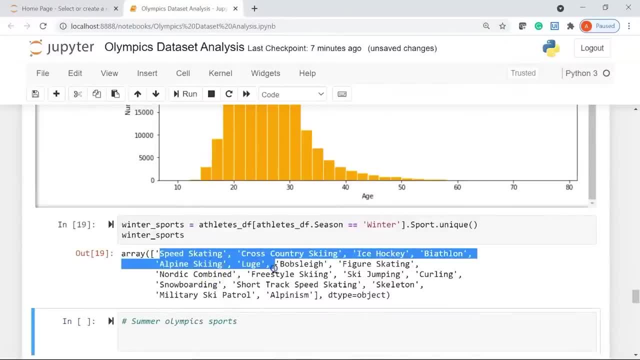 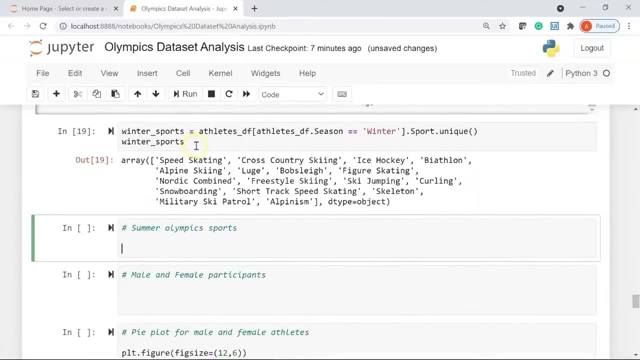 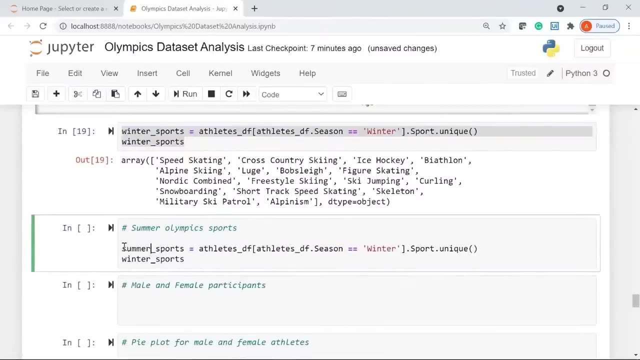 different winter sports that are held during the winter olympics. similarly, let's see for summer olympics. what i am going to do here is i will just copy this cell of code and we will edit the variables. i will say: summer. underscore- sports athletes. underscore df remains the same. 20 to 30. you can see here- so early 20s, we have maximum number of athletes participating in the olympics. we also have a few athletes who are beyond 40 years of age. you can see here we have a few athletes even closer to 60 also. 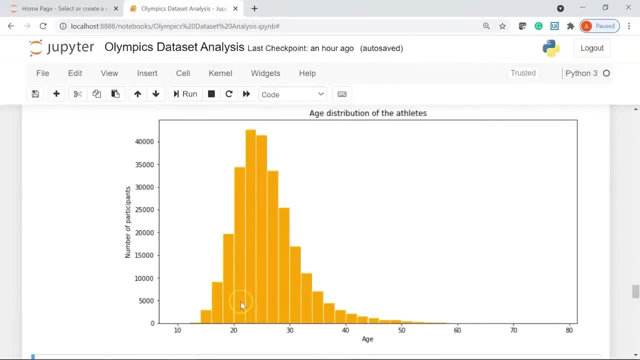 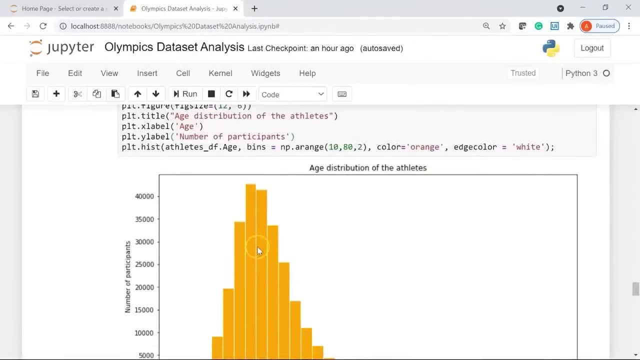 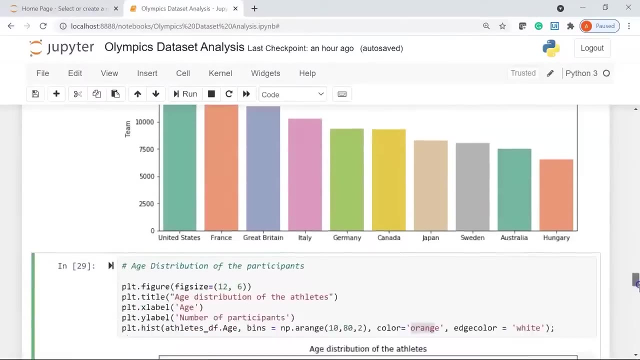 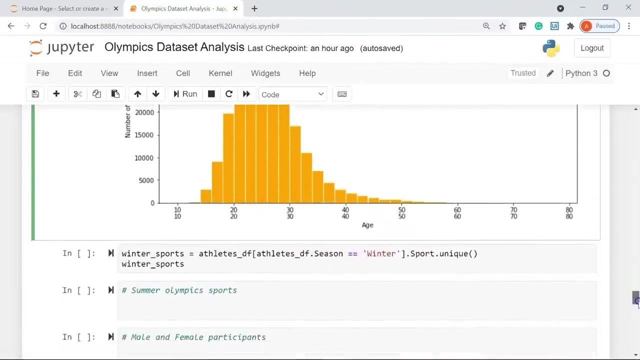 and similarly, we have a few athletes who are under 18 years of age. alright now. you can see here the bins. we had taken orange color, so all the bars are represented in orange color and the edge, you can see here, we have the white color. alright, now moving ahead. 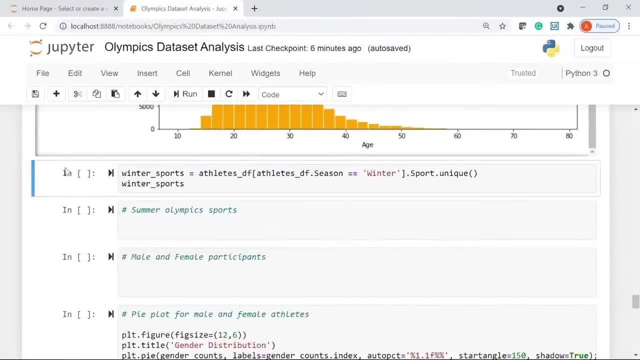 now in the initial slides of the video, we discussed the summer and winter olympic games. let's look at the different sporting events that are part of the summer and winter olympic games. just to give you a heads up, the winter olympic games are held once every 4 years for. 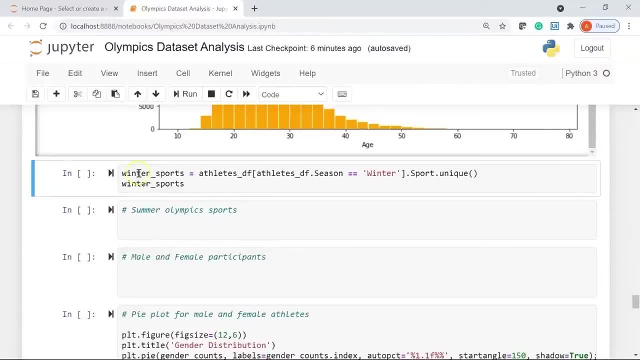 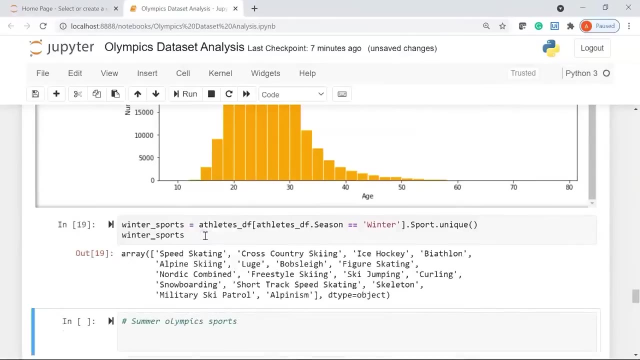 sports practiced on snow and ice. so here i have my variable name: winter underscore sports. so i am extracting for season equal to equal to winter and i am going to display only the unique values. now let me run this cell. ok, so we can see here these are. 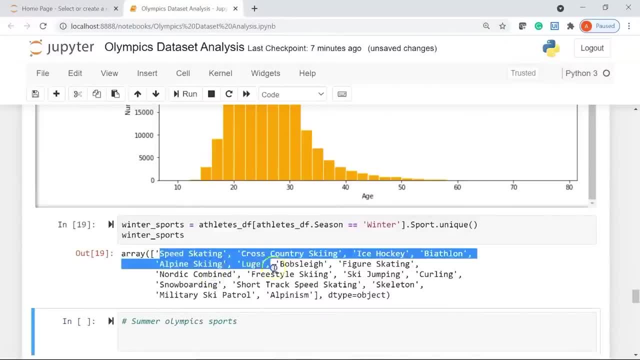 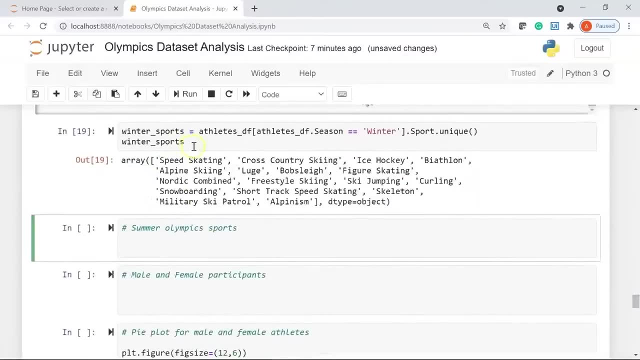 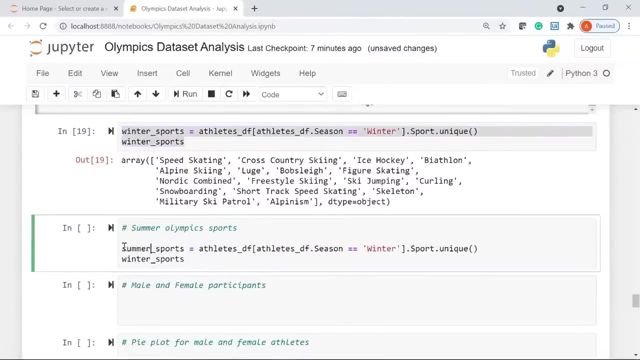 the different winter sports that are held during the winter olympics. similarly, let's see for summer olympics. so what i am going to do here is i will just copy this cell of code and will edit the variables. i will say summer underscore sports athletes. 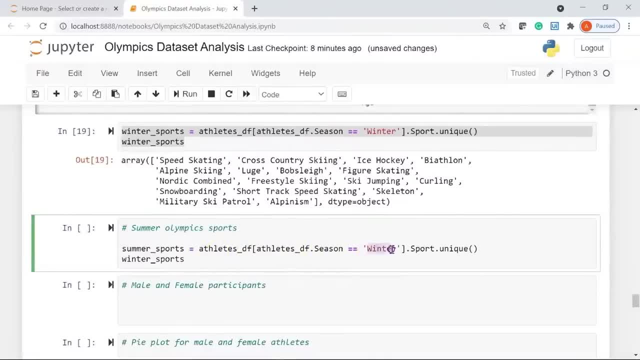 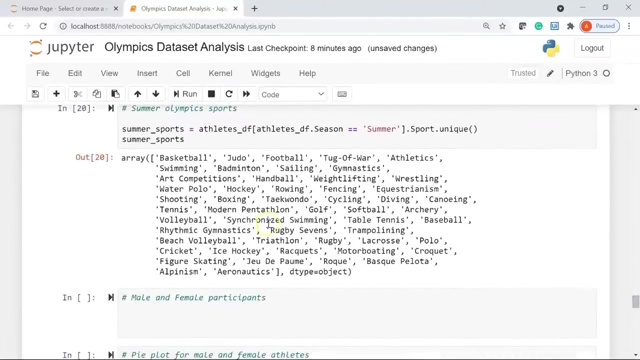 underscore df remains the same. here season we will change it to summer dot sport. dot unique remains the same and here i will say summer underscore sports. this should be small now. let's run it there you go. so here you can see we have more number of olympic sports that. 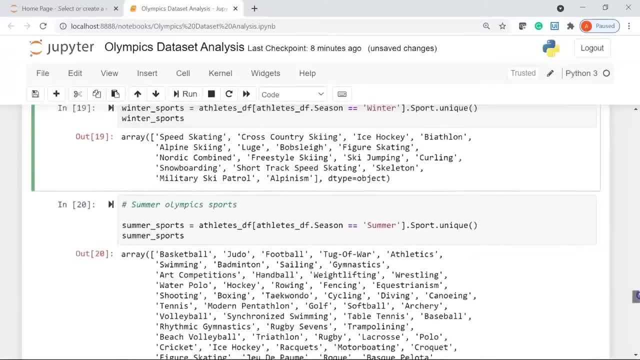 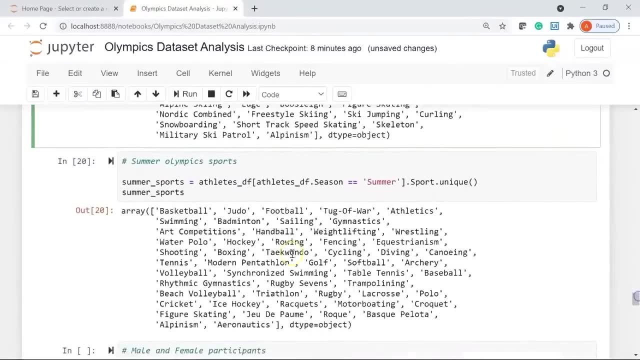 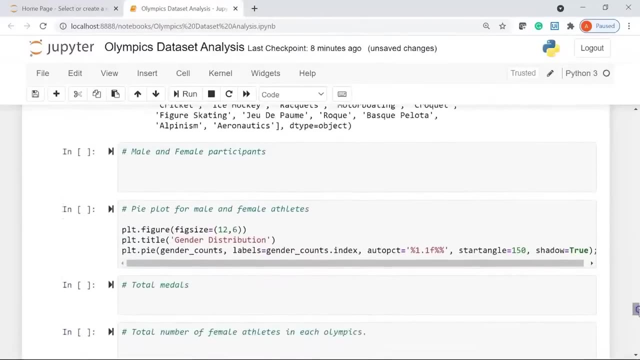 are held during the summer olympics compared to winter olympics. so these are the sports that are played on snow and ice and these are the sports that are played during summer. moving ahead, now it's time to analyze the total number of male and female participants who have taken. 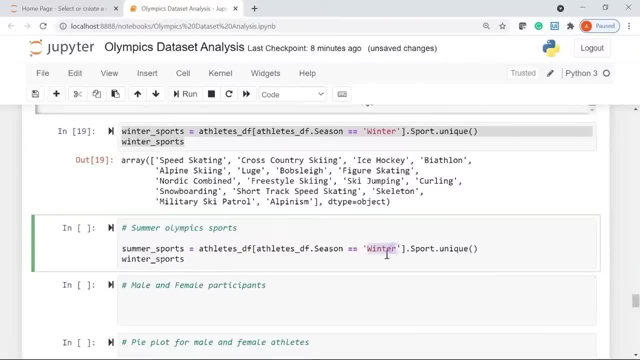 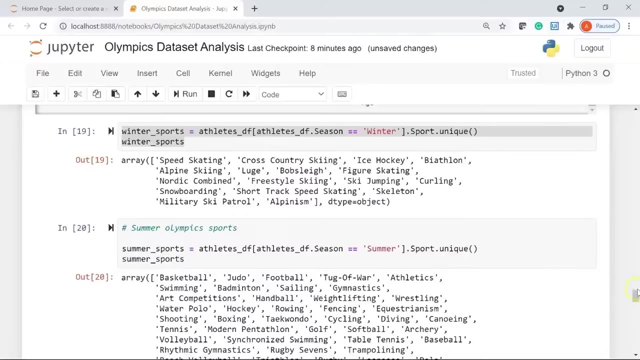 here season, we will change it to summer dot sport. dot unique remains the same, and here i will say summer underscore sports. this should be small now let's run it there you go. so here you can see we have more number of olympic sports that are: 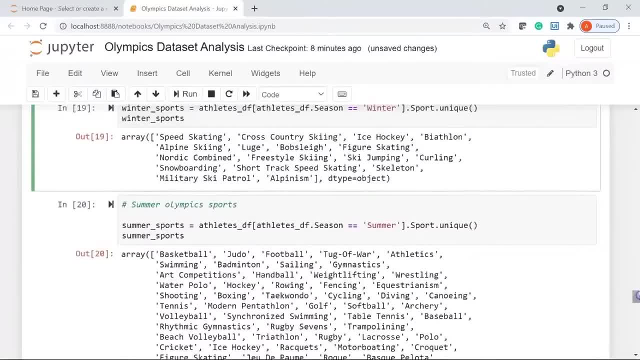 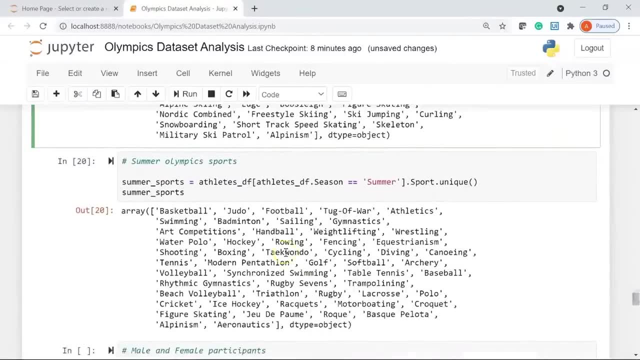 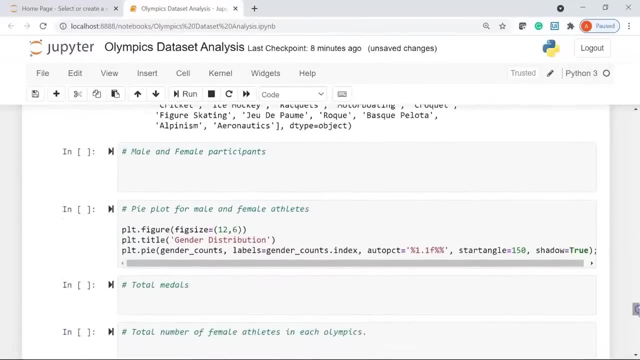 held during the summer olympics compared to winter olympics. so these are the sports that are played on snow and ice and these are the sports that are played during summer. moving ahead, now it's time to analyze the total number of male and female participants who have taken part. 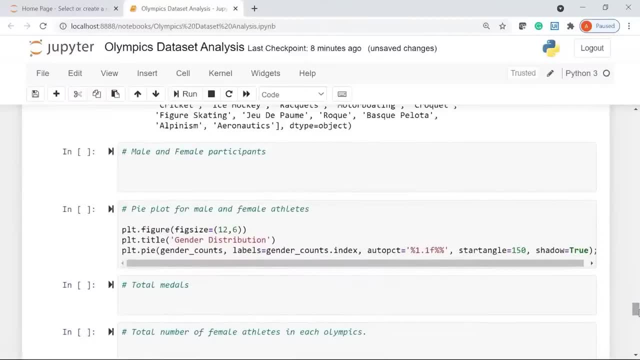 in different games since 1896 till 2016, rio olympics. alright, so i will say gender: underscore counts, which is my variable name. i will use my data frame, that is athletes. underscore df dot, my variable name. that is sex dot. value: underscore counts. and then 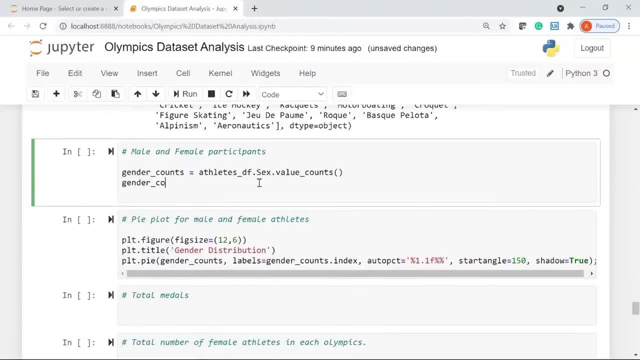 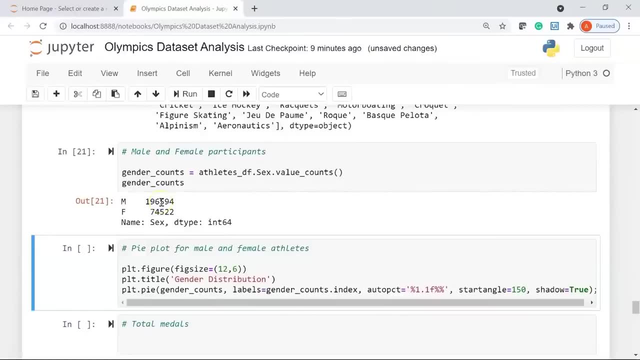 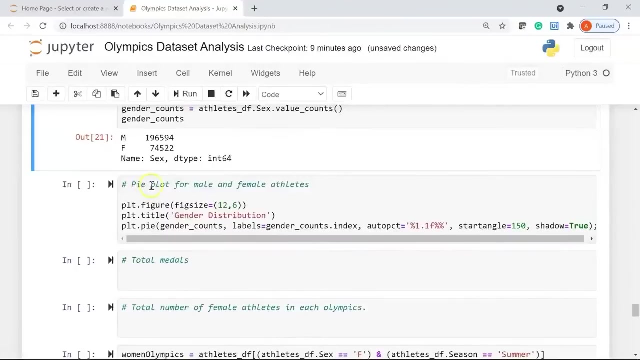 we are going to print gender underscore counts. let's run this. there you go. so since the inception of olympics, we have more number of male participants than female participants. now, here, in this current cell, you can see we are trying to plot a pie chart for. 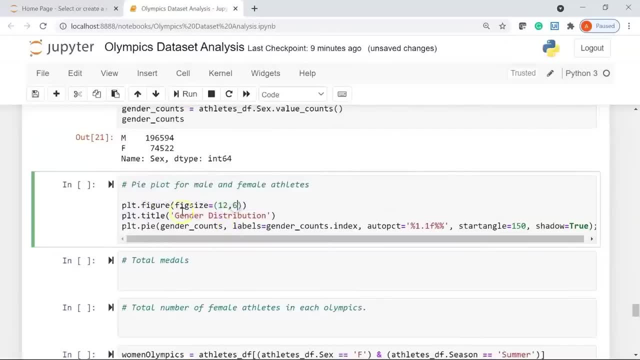 male and female athletes. so i have given my figure size, then i have my title as gender distribution. i am using the matplotlib library and the pie function. i am using the variable gender counts that we used here. then i am giving my labels as gender underscore counts: dot index. 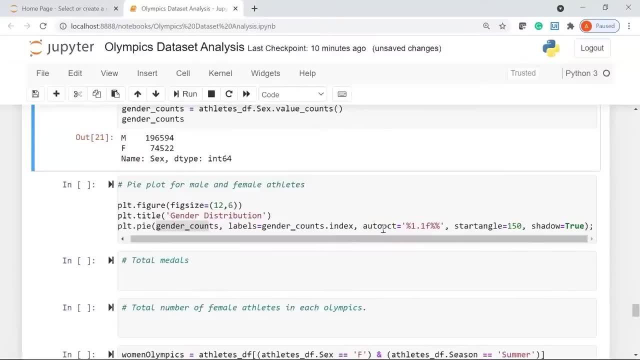 now i am using this auto pct. the auto pct parameter enables you to display the percent value using python string formatting. so this is my string formatting that i have used, and i am initialized my start angle for the pie chart as 150 degrees and i am also giving shadow. 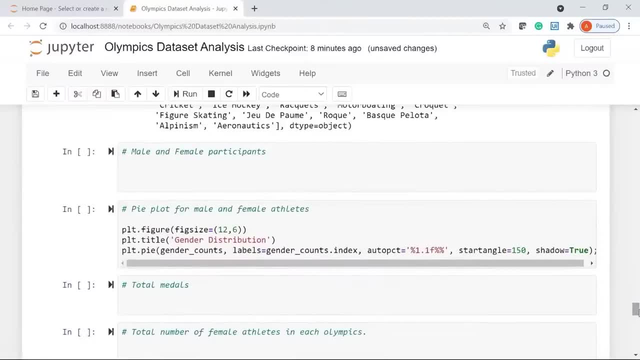 part in different games since 1896 till 2016, rio olympics. alright, so i will say gender: underscore counts, which is my variable name. i will use my data frame. that is athletes. underscore df dot, my variable name. that is sex dot. value: underscore counts. 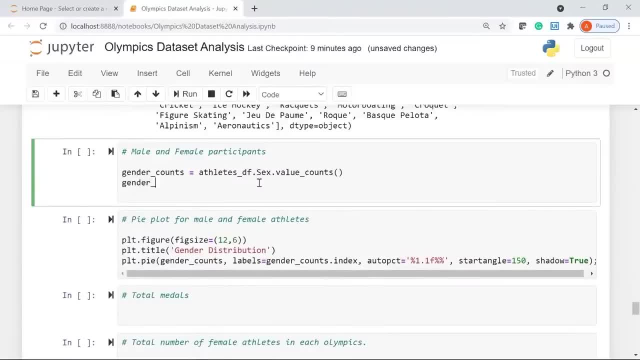 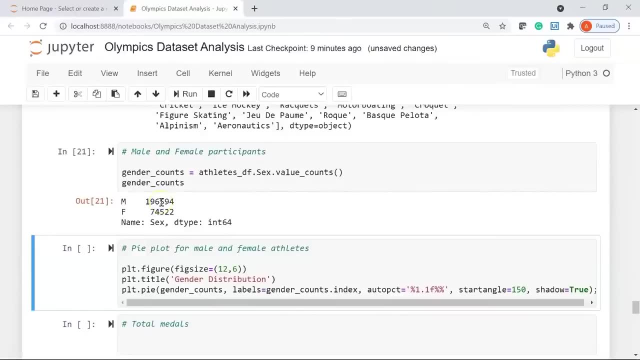 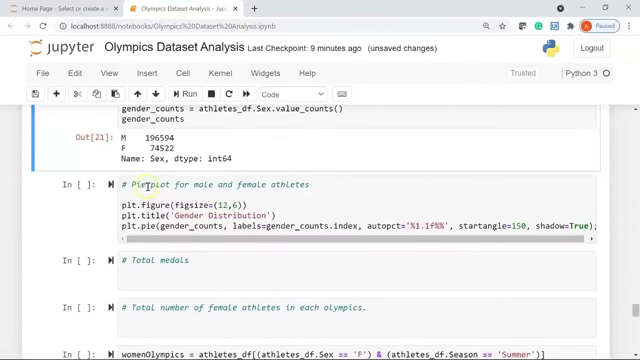 and then we are going to print gender underscore counts. let's run this. there you go. so since the inception of olympics, we have more number of male participants than female participants. now, here in this current cell, you can see we are trying to plot a pie chart. 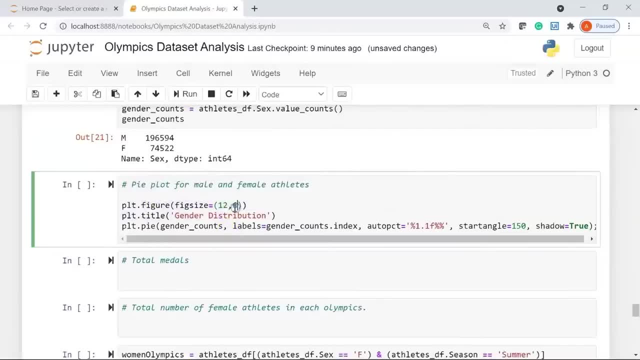 for male and female athletes. so i have given my figure size and i have my title as gender distribution. i am using the matplotlib and the pi function. i am using the variable gender counts that we used here. then i am giving my labels as gender underscore counts dot. 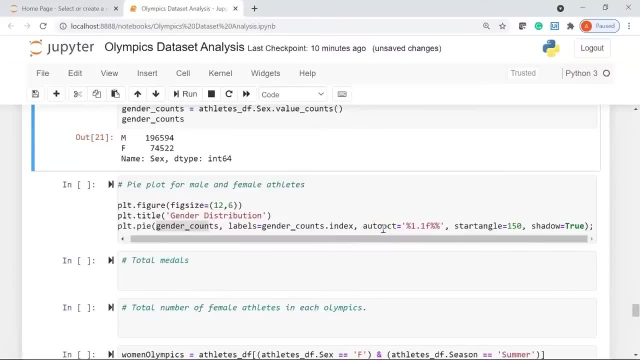 index. now i am using this auto pct. the auto pct parameter enables you to display the percent value using python string formatting. so this is my string formatting that i have used, and i am initialized my start angle for the pie chart as 150 degrees and i am also giving shadow. 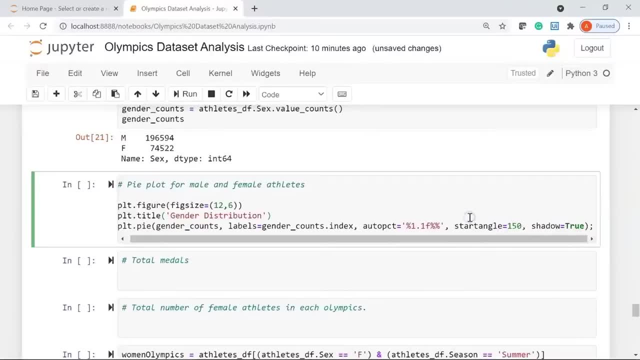 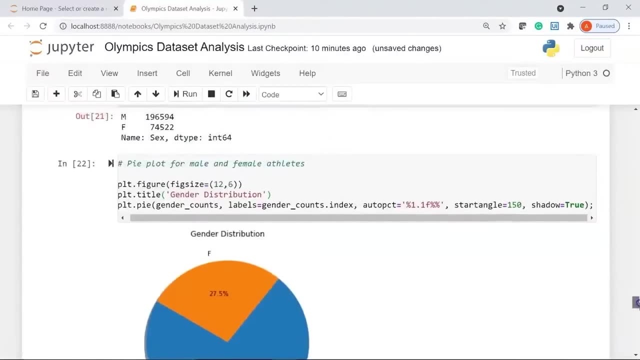 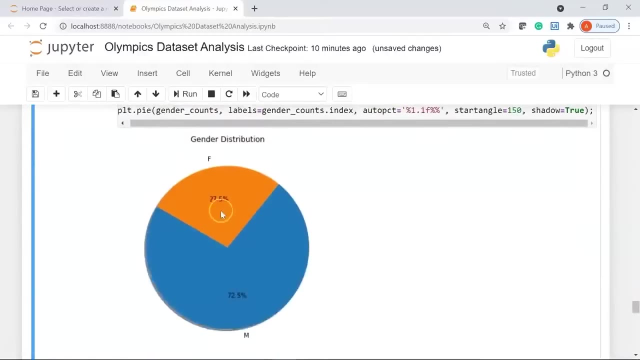 to my pie chart. so i have written shadow equal to true. let's run it alright, so you can see here. this is my pie chart that shows you the distribution of the male and female participation. so for male it is 72.5% for female. so far it is. 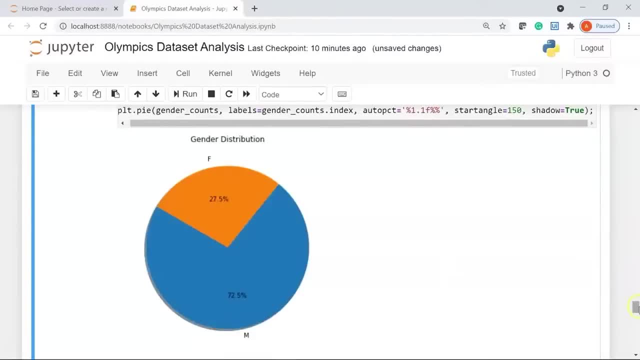 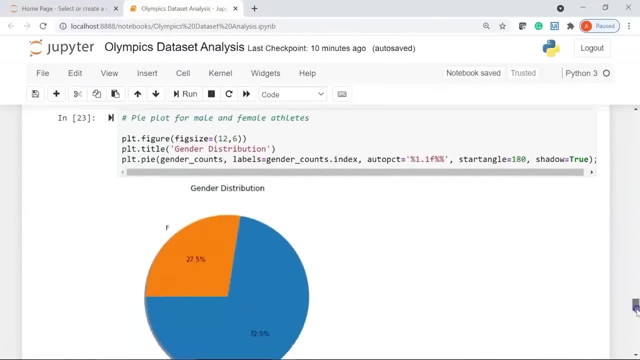 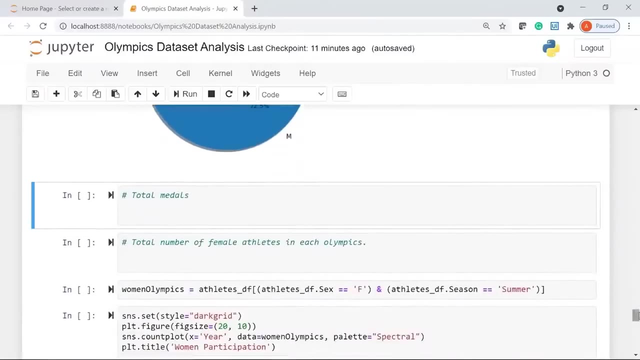 27.5%, as per the dataset that we have. we can change this start angle to, let's say, 180 degree and it will change the pie chart to this direction. cool, now moving ahead. this time we are going to find the total number of medals. 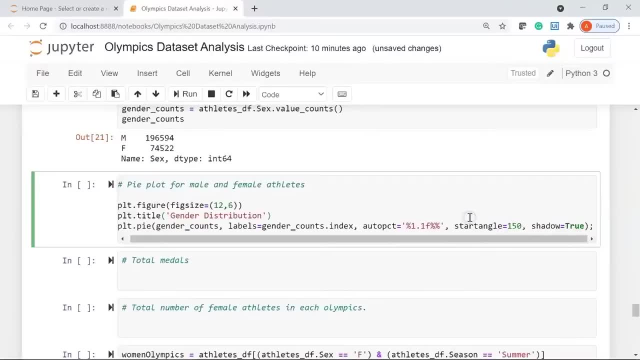 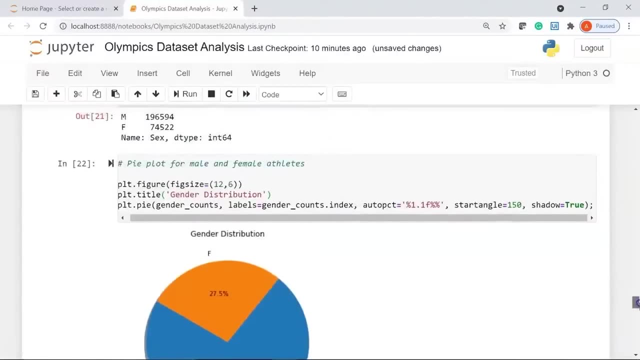 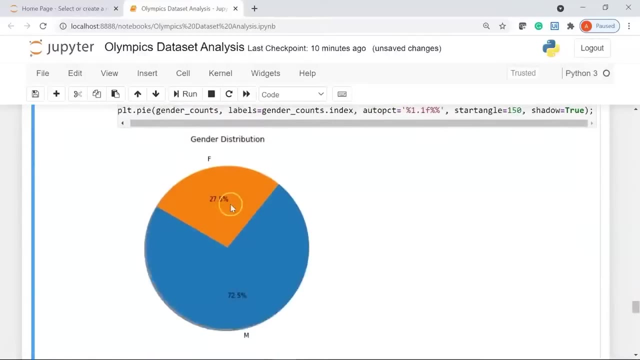 to my pie chart. so i have written shadow equal to true. let's run it alright, so you can see here. this is my pie chart that shows you the distribution of the male and female participation. so for male it is 72.5 percent. for female, so far it is. 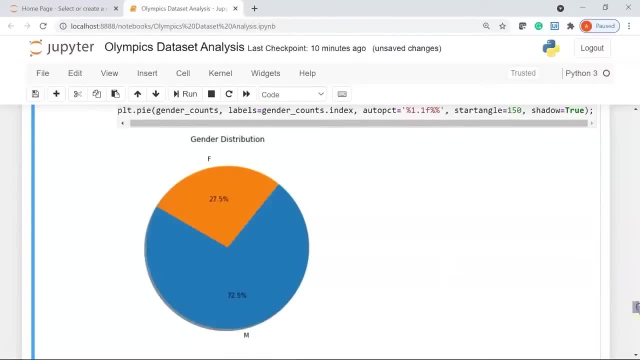 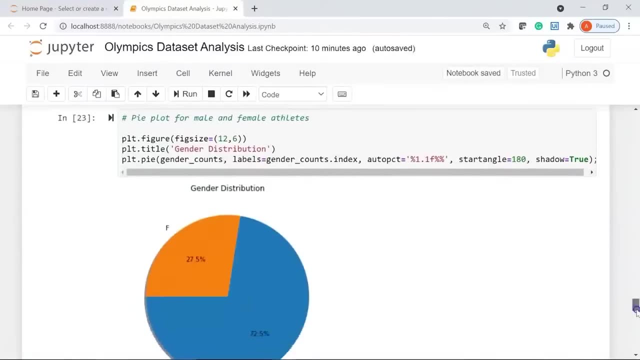 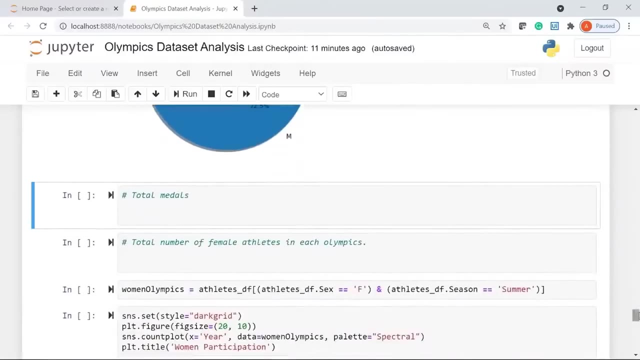 27.5 percent, as per the data set that we have. we can change this start angle to, let's say, 180 degree and it will change the pie chart to this direction. cool, now moving ahead. this time we are going to find the total number of medals. 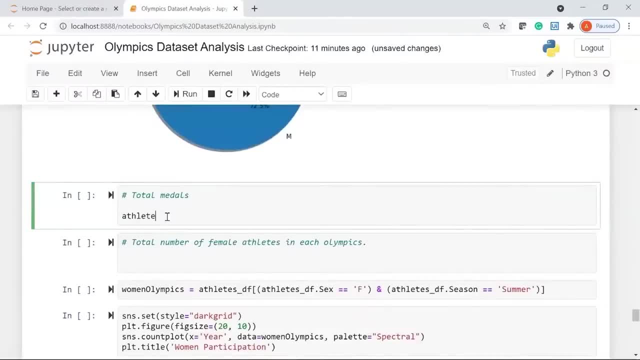 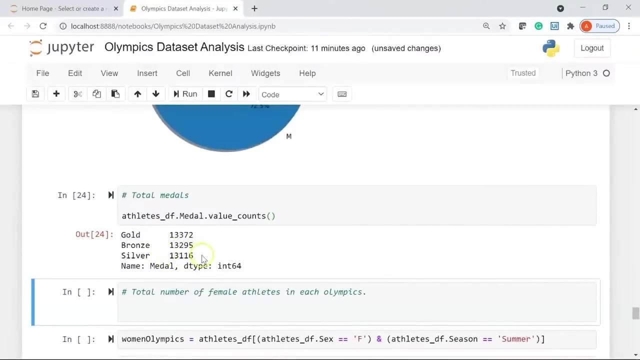 that the athletes have won. so i will use my data frame, athletes, underscore df, dot and then my column that is medal. i will say dot value underscore counts. let's run it. there you go. so you can see the gold medals, the bronze medals and the silver medals are very 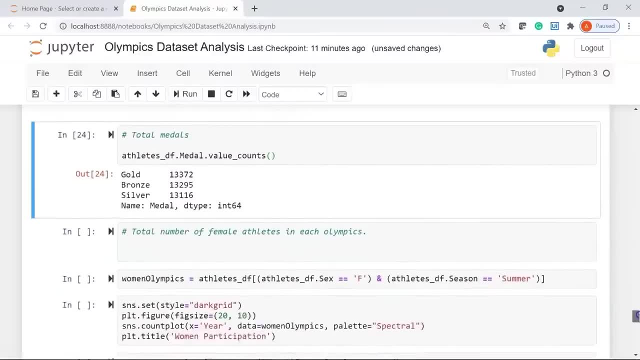 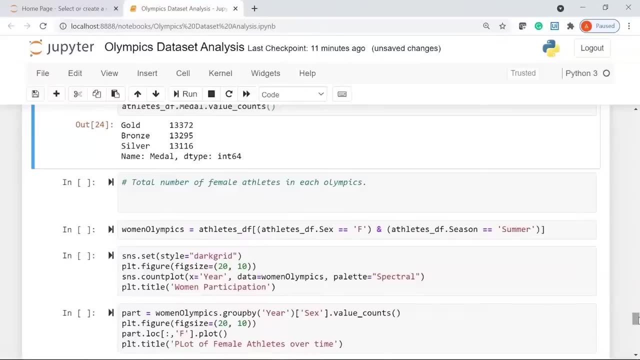 much similar to each other. the numbers are pretty much the same. alright, now it's time to focus on the total female athletes who have taken part in each olympics. so i will create a variable called female underscore participants. i will say equal to and then use my data frame name. 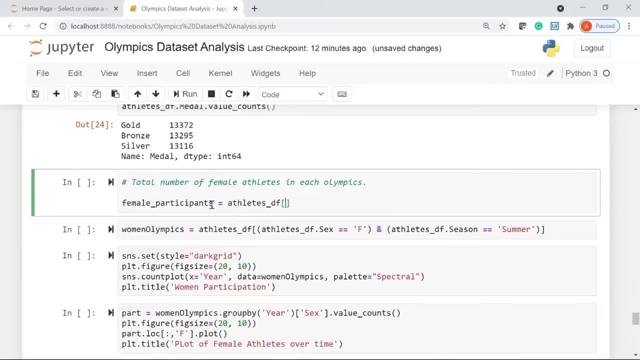 that is, athletes underscore df. using square brackets. i will say: athletes underscore df: dot. the gender should be equal to, equal to female and i will use ampersand. i will say: just copy this, paste it here. i will say: dot. season equal to equal to. we will check for. 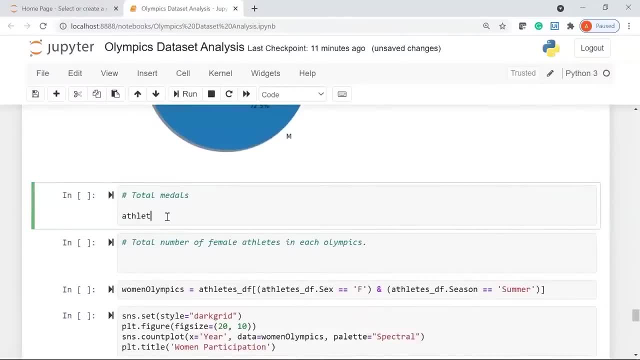 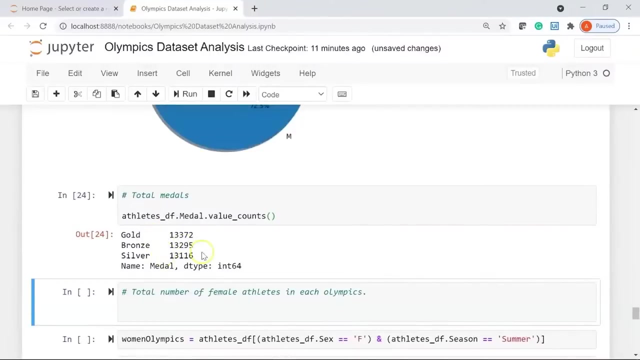 that the athletes have won. so i will use my data frame athletes, underscore df, dot and then my column that is medal. i will say dot value underscore counts. let's run it. there you go. so you can see the gold medals, the bronze medals and the silver medals are. 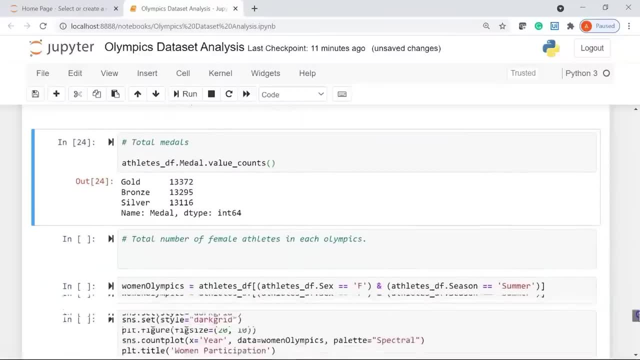 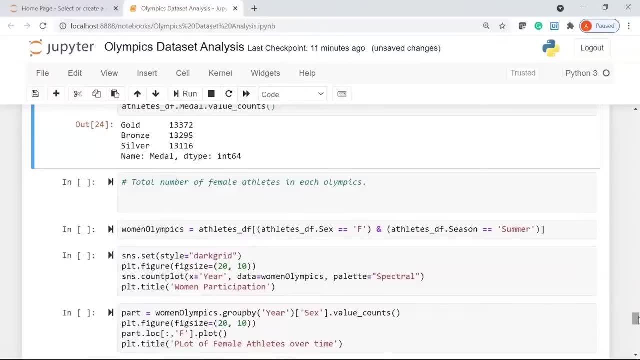 very much similar to each other. the numbers are pretty much the same. alright, now it is time to focus on the total female athletes who have taken part in each olympics. so i will create a variable called female underscore participants. i will say equal to and then use my data frame name. 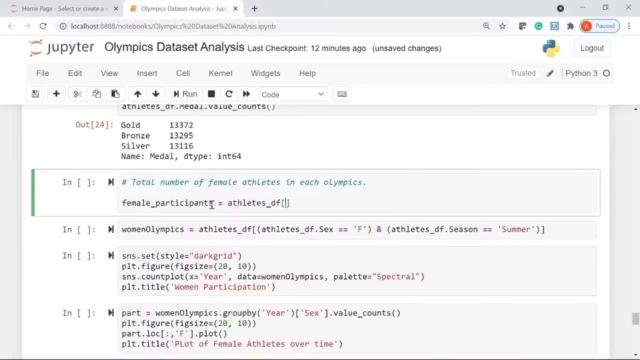 that is, athletes underscore df. using square brackets. i will say: athletes underscore df: dot. the gender should be equal to, equal to female and i will use ampersand. i will say: just copy this, paste it here. i will say: dot. season equal to equal to. we will check. 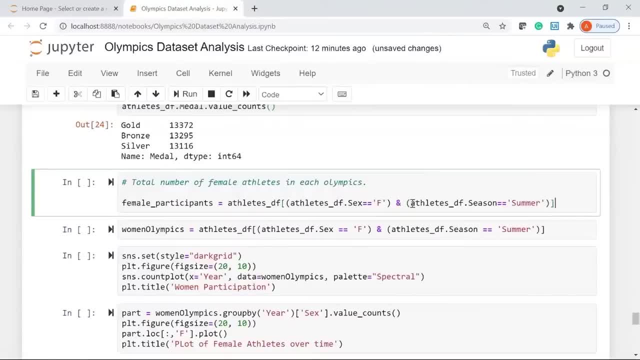 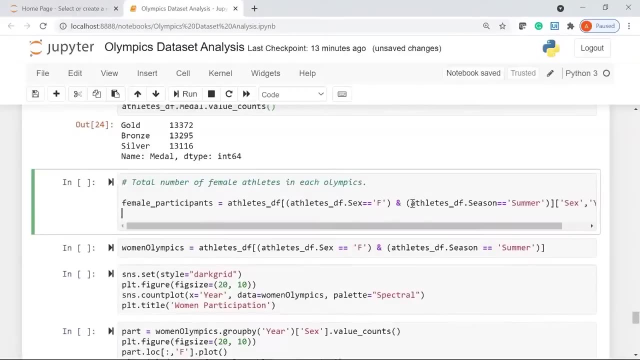 for summer olympics and i want to extract only the gender column. so here it is sex comma, my year column, which is year ok, and then i will say: female underscore participants equal to. i will just copy this, paste it here and then i will use the group by function. 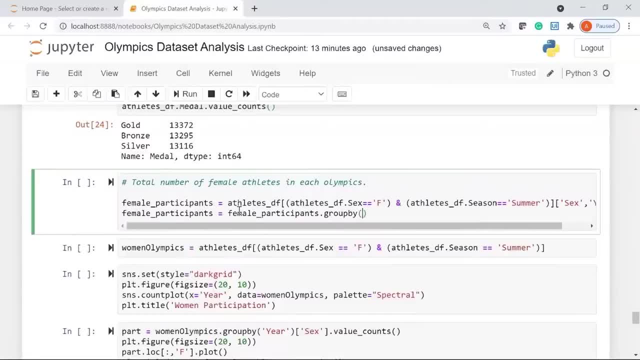 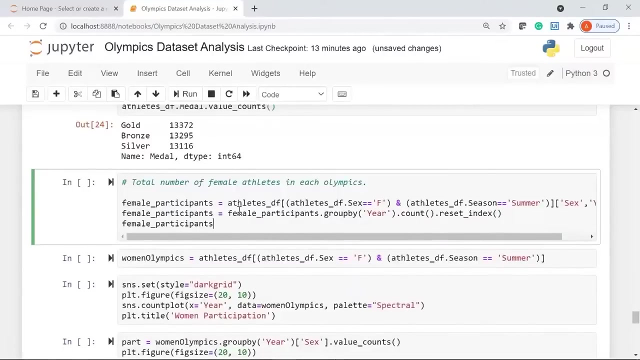 say group by which is part of the pandas library, i will say year and then i want to find the count. i will reset the index, say reset underscore. index is a function and finally we are going to print female underscore participants and let's say the head: alright, 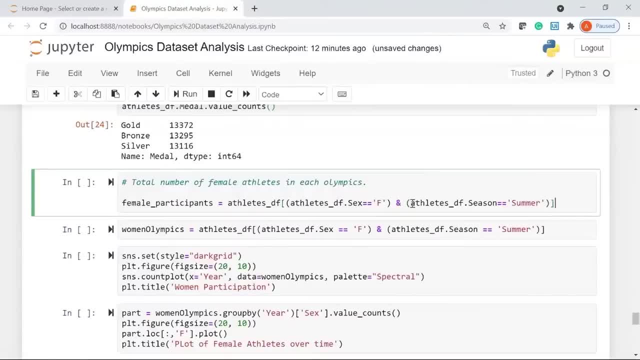 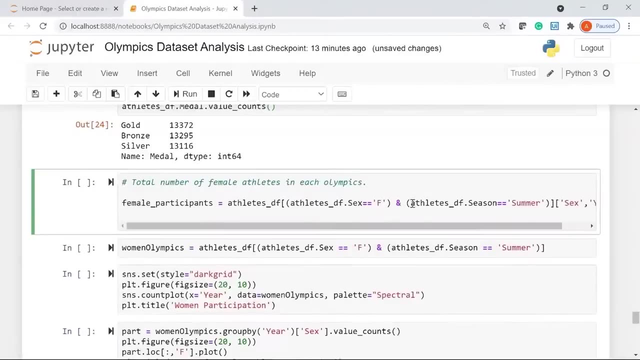 summer olympics and i want to extract only the gender column. so here it is sex comma, my year column, which is year ok, and then i will say: female underscore participants equal to. i will just copy this, paste it here and then i will use the group by function. 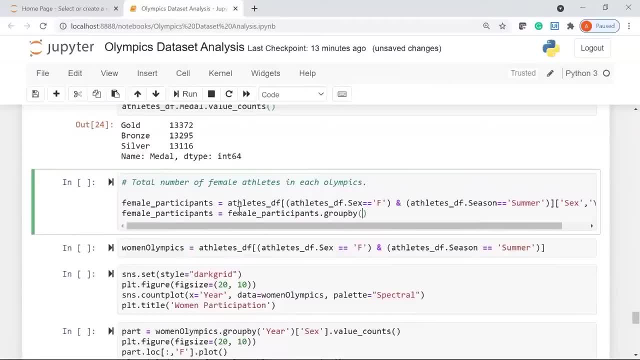 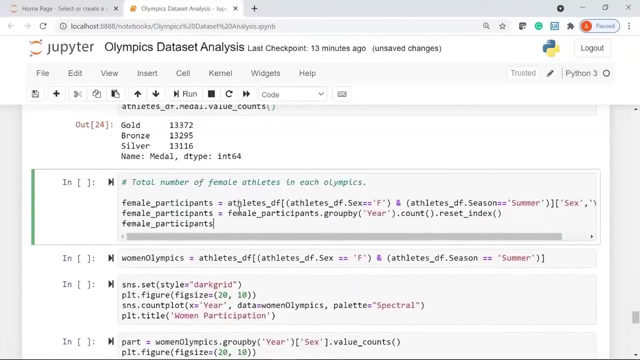 say group by which is part of pandas library, i will say year and then i want to find the count. i will reset the index, say reset underscore. index is a function, and finally we are going to print female underscore participants and let's say the head: alright. so what we are trying to do is 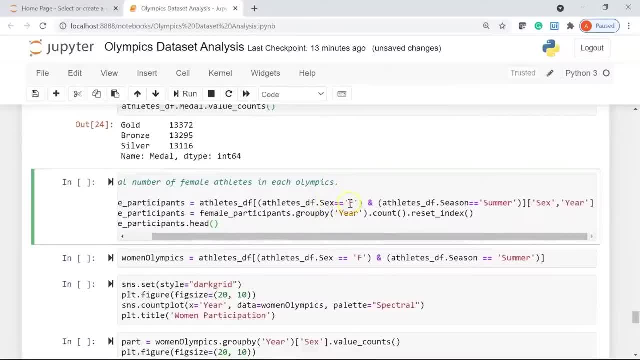 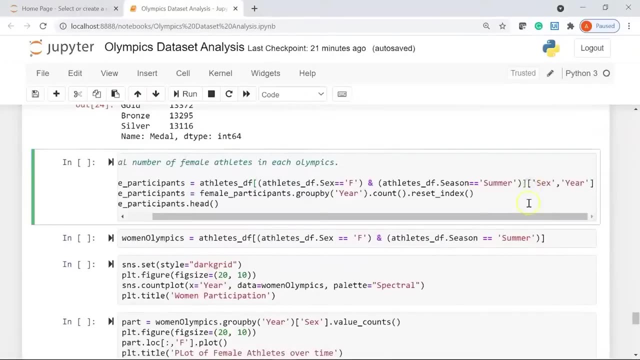 i am trying to filter the data only for the female athletes for summer olympics, and here i am printing the participation based on each year, so i am finding out the count. so here we need to add one more square bracket. alright, now we will run it and see the result. 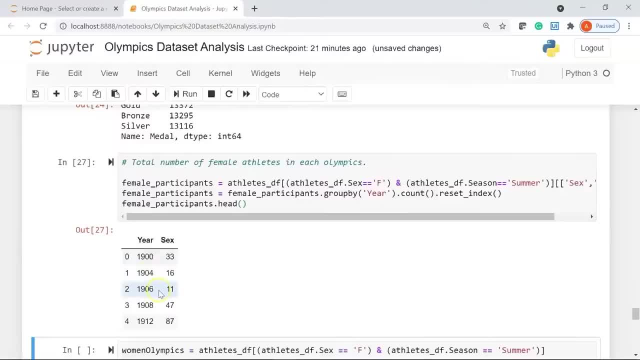 there you go, so you can see here from 1900, all these years you can see the female participation. let me change it to tail so that we have the recent data of the olympics. you can see it here for the beijing olympics. 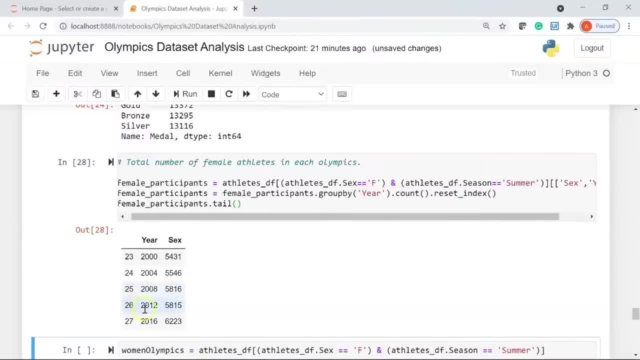 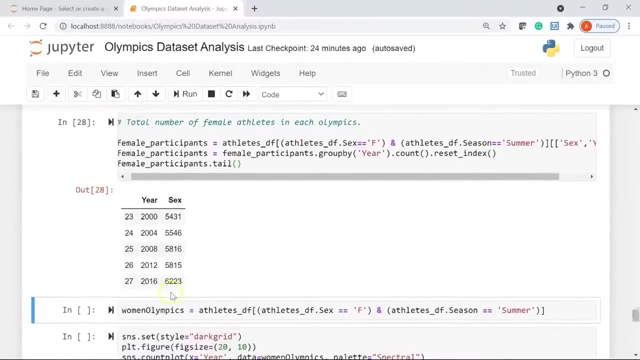 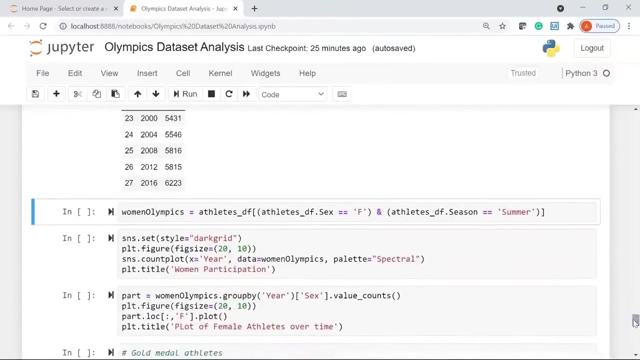 5816 women athletes participated in 2012 london olympics. we had 5815 olympics. similarly, for the 2016 rio olympics, we had more participation than the olympics, so 6223 women athletes had participated. alright, now here. 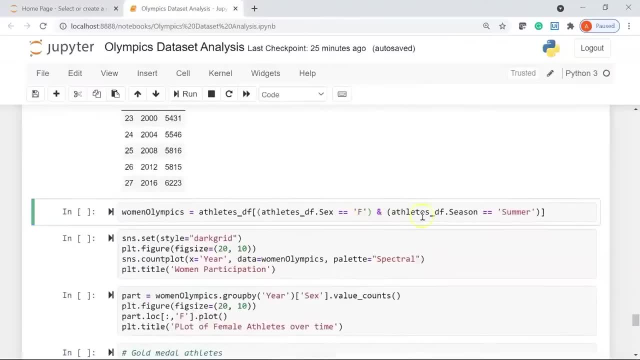 this is another way in which you can filter your data for female athletes. so i am using two parameters: my gender should be equal to female and season is summer olympics. let me just run it. i have stored it in a variable called women- olympics. 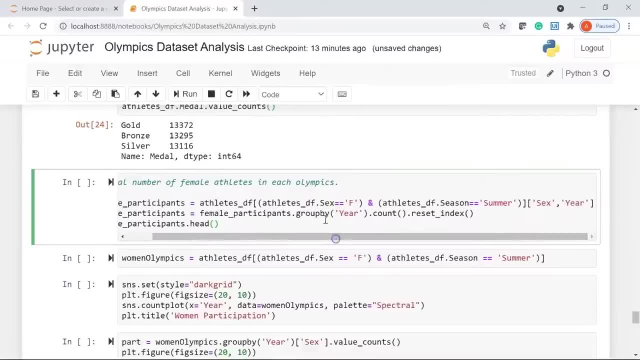 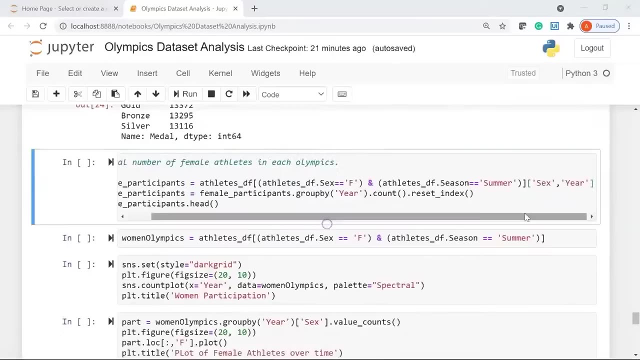 so what we are trying to do is i am trying to filter my data only for the female athletes for summer olympics, and here i am printing the participation based on each year, so i am finding out the count. so here we need to add one more square. 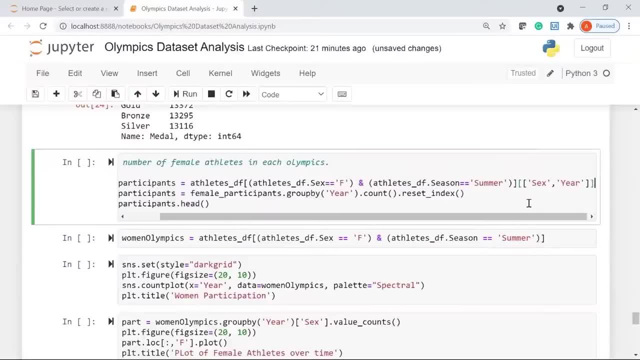 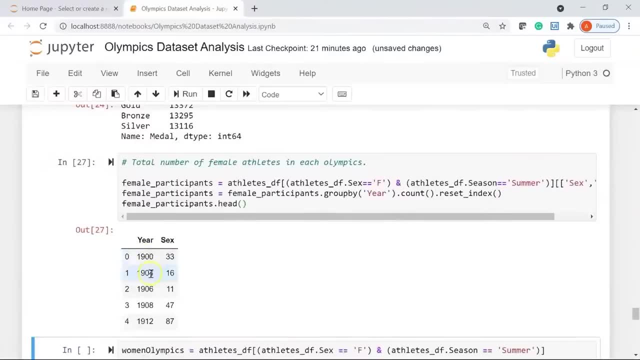 bracket. alright, now we will run it and see the result. there you go, so you can see here, from 1900, 1904, all these years, you can see the female participation. let me change it to tail so that we have the recent data of the olympics. 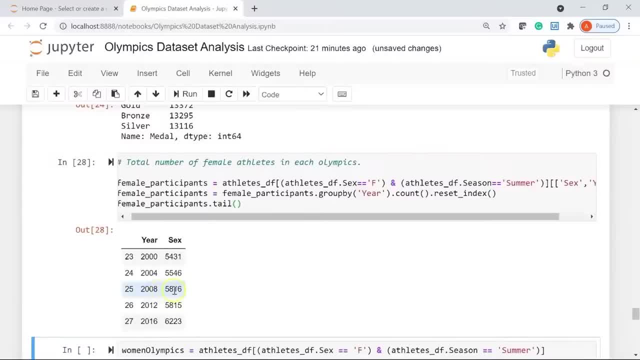 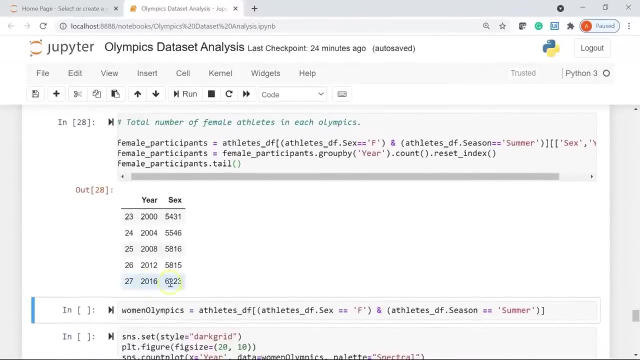 you can see it here. for the beijing olympics, 5816 female athletes participated. in 2012 london olympics, we had 5815 olympics. similarly, for the 2016 rio olympics, we had more participation than the london olympics. so 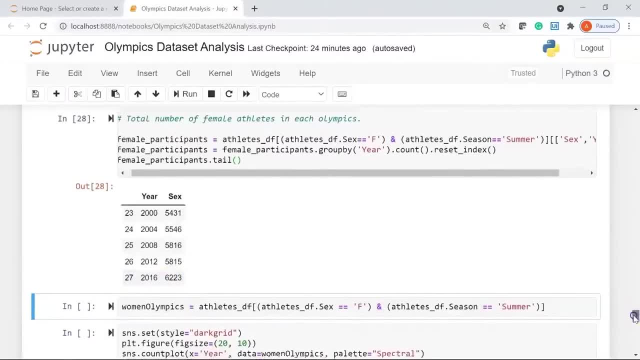 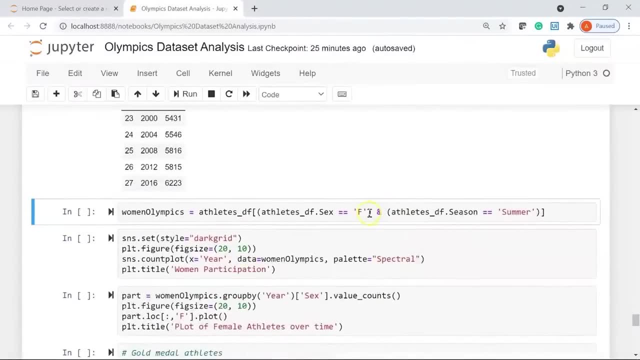 6223 women athletes had participated. alright, now here, this is another way in which you can filter your data for female athletes. so i am using two parameters: my gender should be equal to female and season is summer olympics. let me just run it. i have. 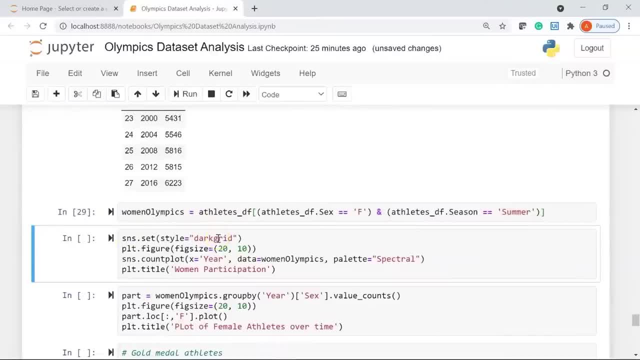 stored it in a variable called women olympics. now here i am trying to find a count plot, or i am trying to create a count plot using my sns library. i have set my style to dark grid, then my figure size. i have given as 20,10 my count. 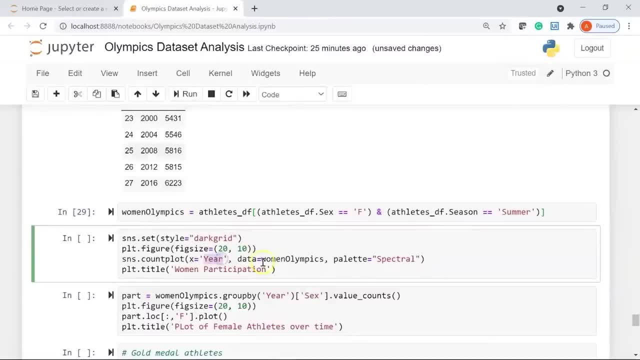 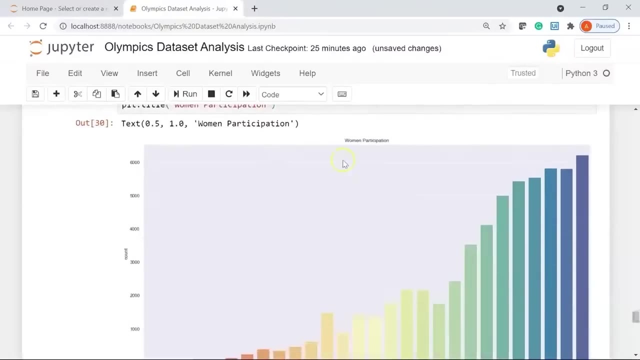 plot will have the x axis as year. the data is women olympics and palette i am using as spectral and then i have given a title: women participation. let's run and see the output. there you go. if i scroll down, you can see on the top. 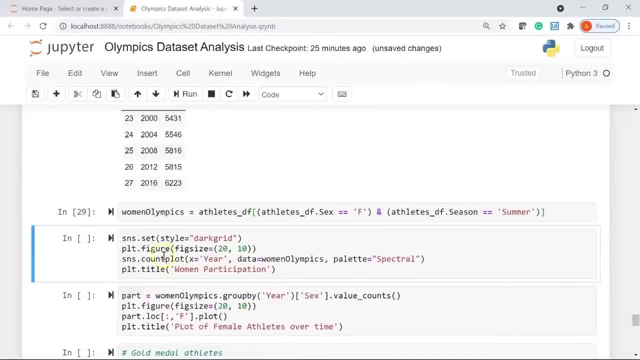 now here i am trying to find a count plot, or i am trying to create a count plot using my seaborn sns library. i have set my style to dark grid. then my figure size i have given as 20 comma 10. my count plot will have the x-axis. 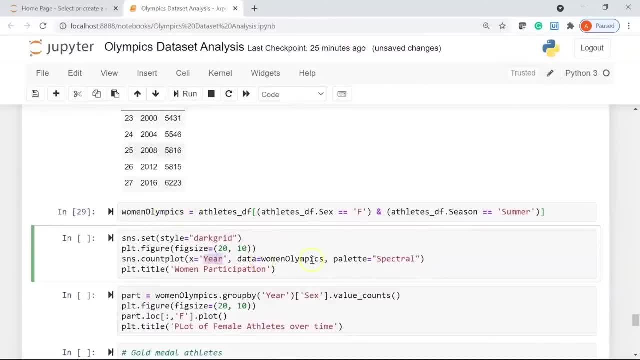 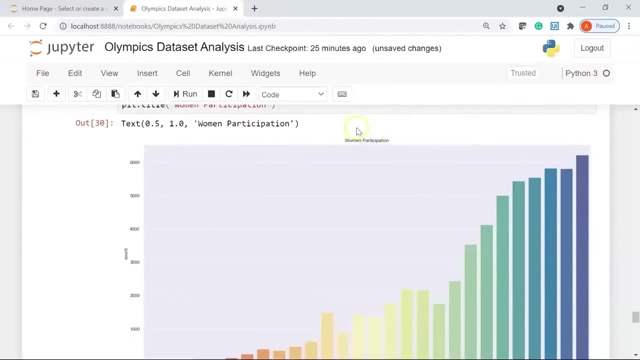 as year. the data is women olympics and palette i am using as spectral and then i have given a title: women participation. let's run and see the output. there you go. if i scroll down, you can see on the top i have the title for my count. 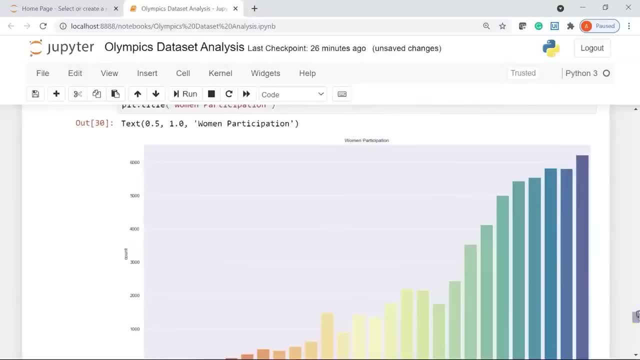 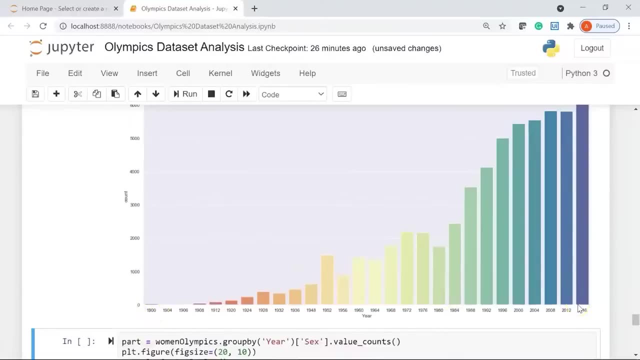 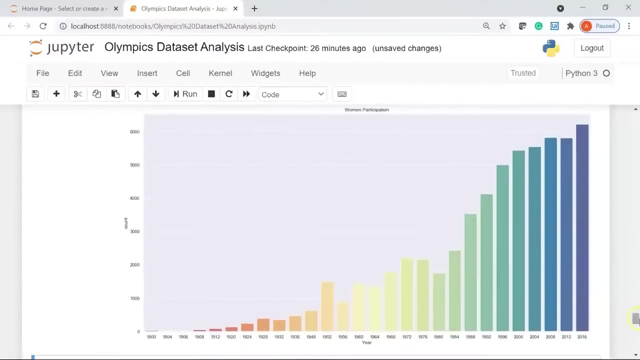 plot which says women participation, and on the y-axis i have the count and at the bottom you can see the different year values from 1900 till 2016. and 2016 had the highest number of female participation. cool, let me scroll down. so in this cell of code we are: 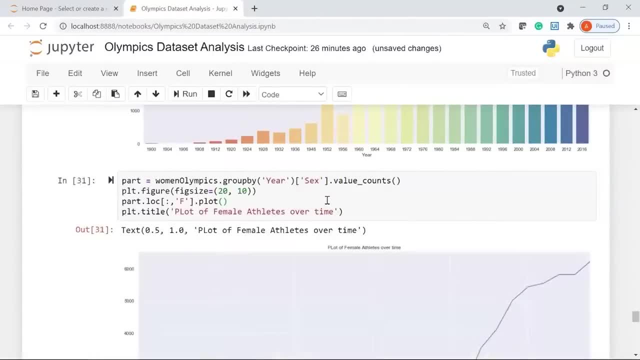 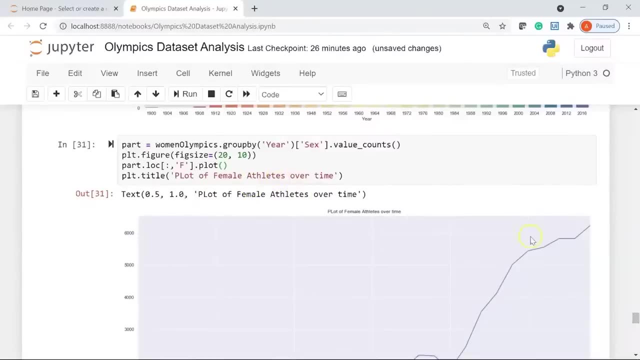 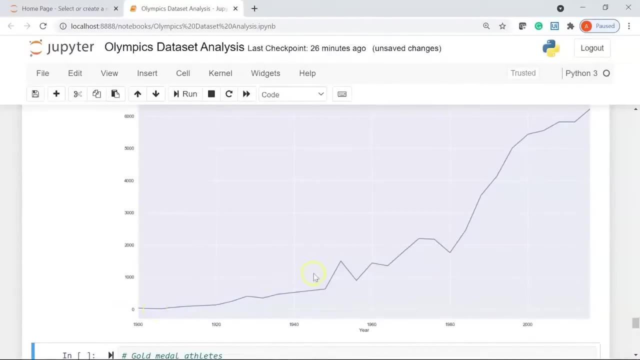 trying to plot a line graph, let me run it and show you the output. so this line graph shows the trend which says plot for female athletes over time. so here you can see the line graph. so gradually the women participation has increased in olympics since its inception. 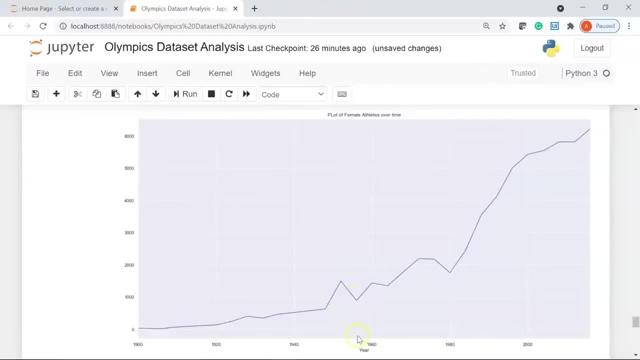 there was a slight decrease here. this is around 1950s and again you can see here there is a decrease with the women participation in 1980. but since then, since 1980, there has been continuous increase in the participation of female athlete numbers cool. 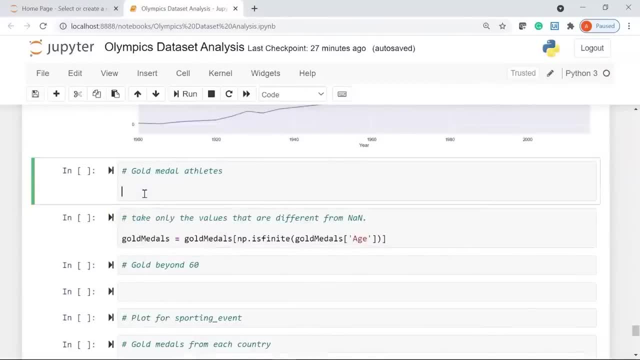 now coming to the next section of our analysis. now we are going to filter the data to see the details of the athletes who have won gold medals. so i will create a variable called gold medals, so equal to. i will use my data frame as athletes. underscore df. 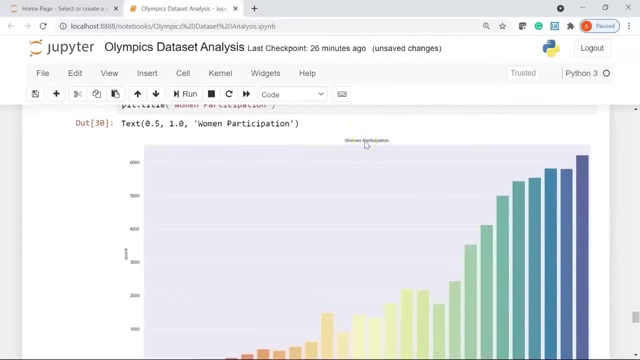 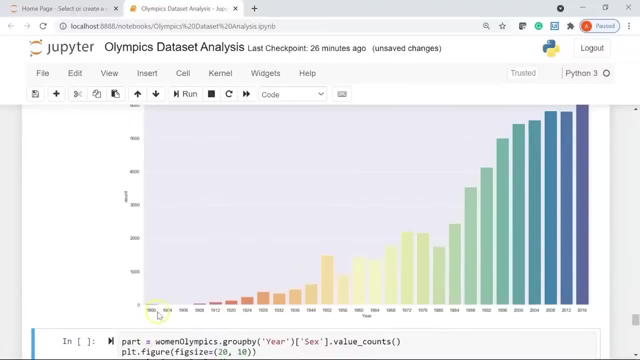 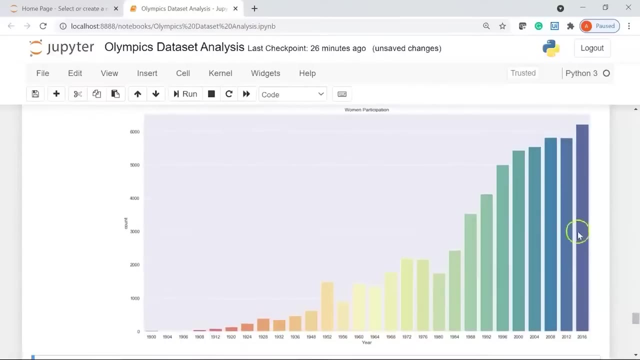 i have the title for my count plot, which says women participation, and on the y axis i have the count and at the bottom you can see the different year values from 1900 till 2016, and 2016 had the highest number of female participation. 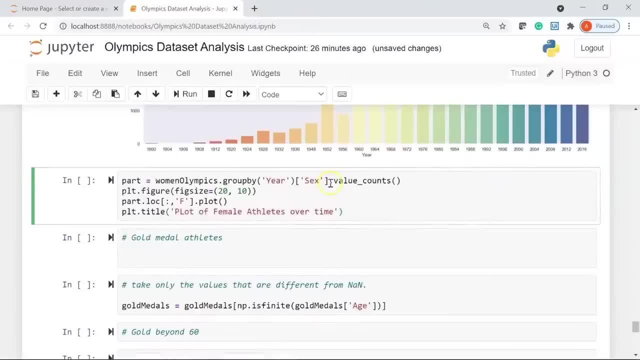 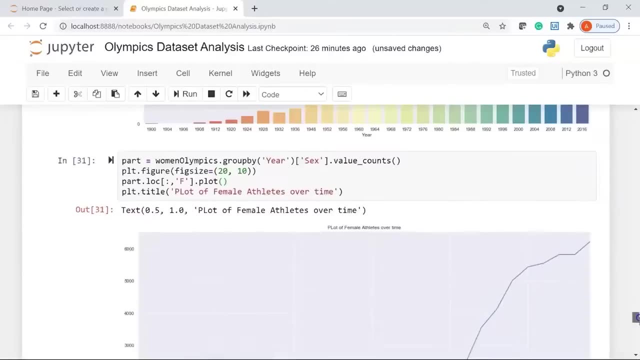 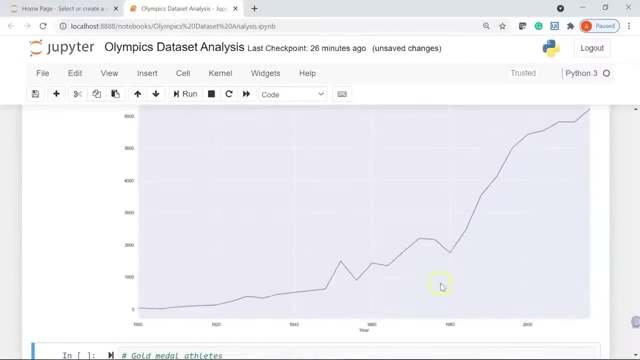 cool, let me scroll down. so in this cell of code we are trying to plot a line graph. let me run it and show you the output. so this line graph shows the trend which says plot for female athletes over time. so here you can see the line graph. 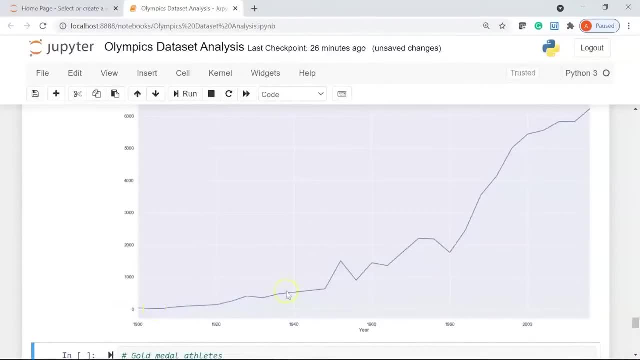 so gradually the women participation has increased in olympics since its inception. there was a slight decrease here. this is around 1950s and again you can see here there is a decrease with the women participation in 1980. but since then, since 1980, there has been continuous. 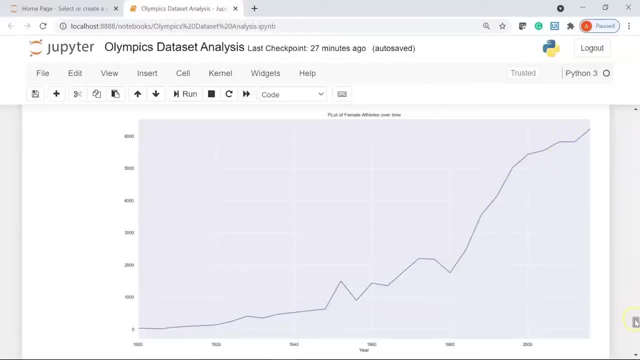 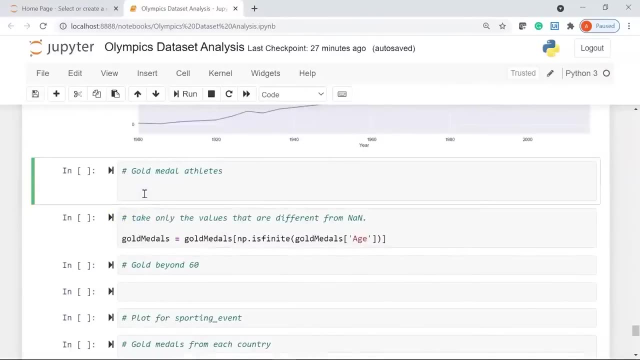 increase in the participation of female athlete numbers- cool. now coming to the next section of our analysis. now we are going to filter the data to see the details of the athletes who have won gold medals, so i will create a variable called gold medals. it's equal to. i will use: 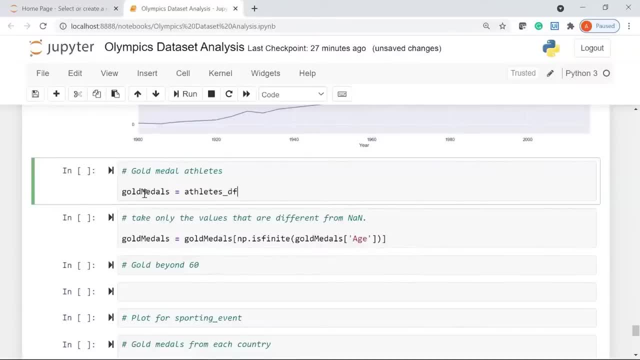 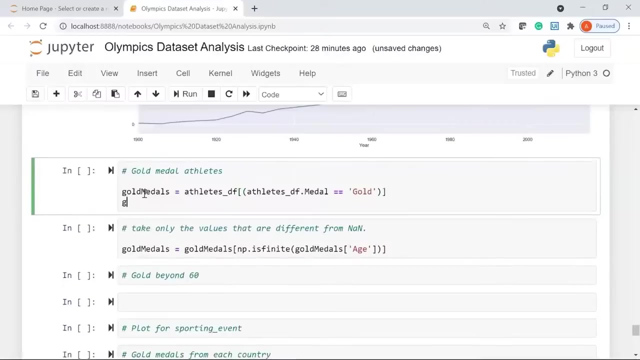 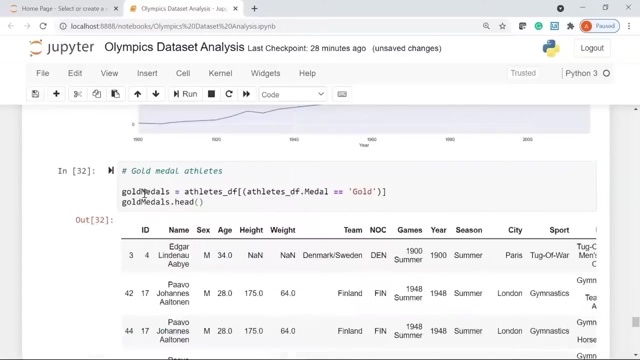 my data frame as athletes underscore df and within parenthesis i will use my data frame name, which is athletes underscore df- dot. i will use the condition medal equal to, equal to, and my value would be gold. next i am going to say gold medals- dot. head, let's run it. 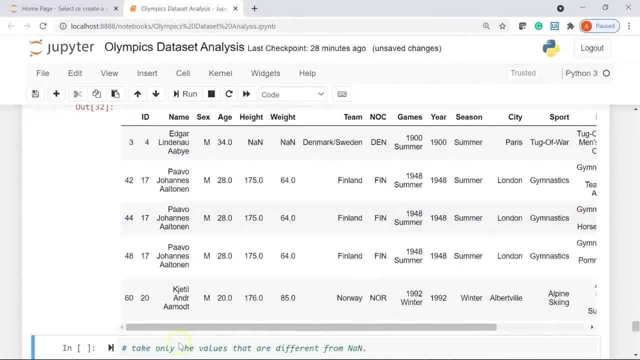 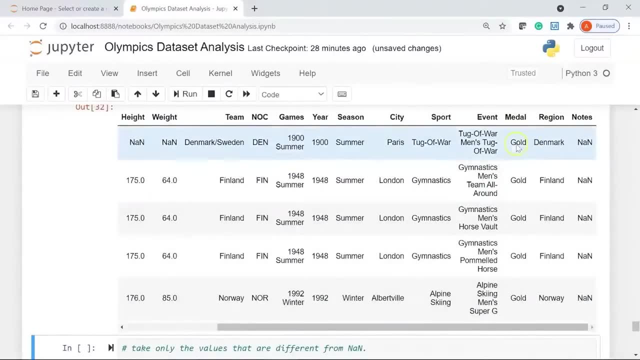 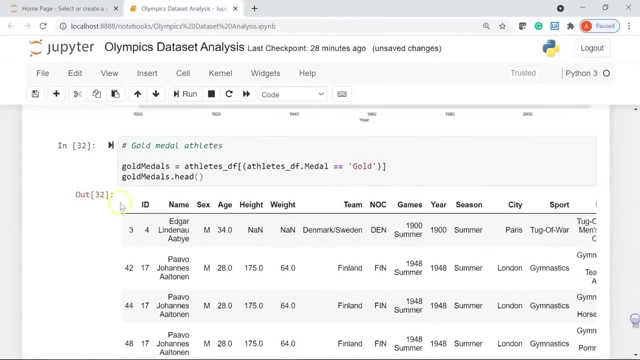 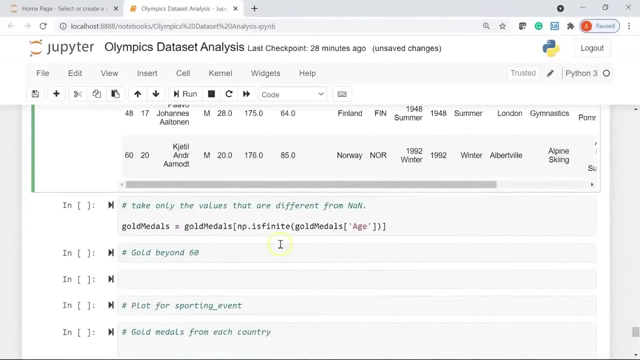 there you go. so here we have the top five rows of the athletes who have won a gold medal. you can see all the records have medal as gold. now we are going to use this subset of the data and perform some more analysis, so here i want to take only the values. 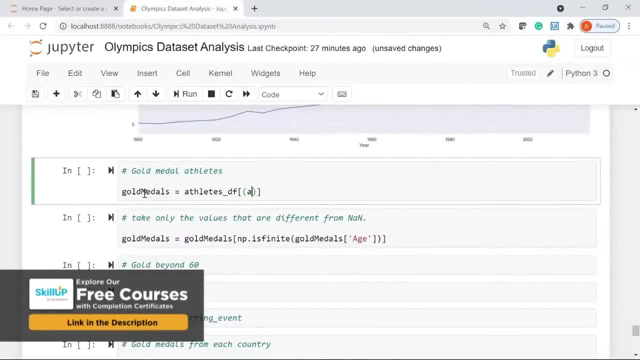 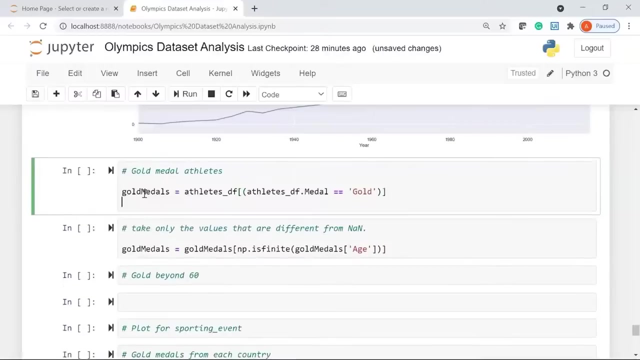 and, within parenthesis, i will use my data frame name, which is athletes. underscore df, dot. i will use the condition medal equal to, equal to, and my value would be gold. next, i am going to say: gold medals, dot head. let's run it there. you go, so here. 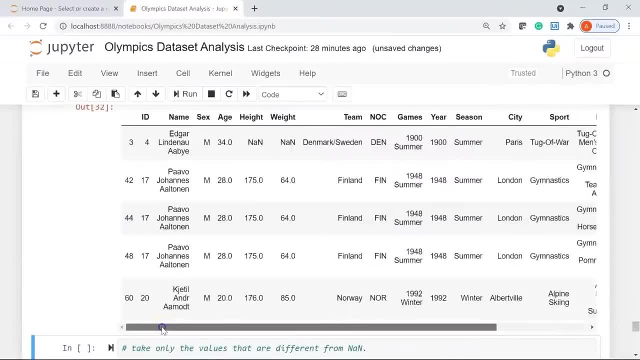 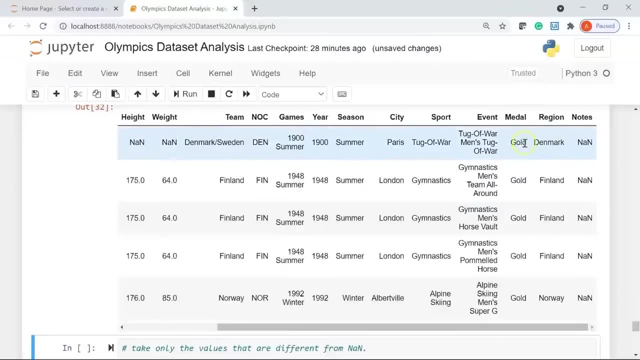 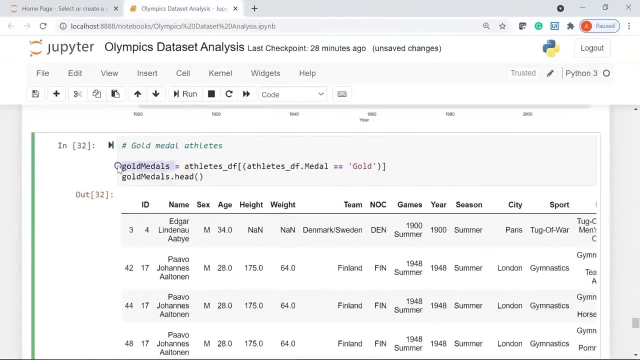 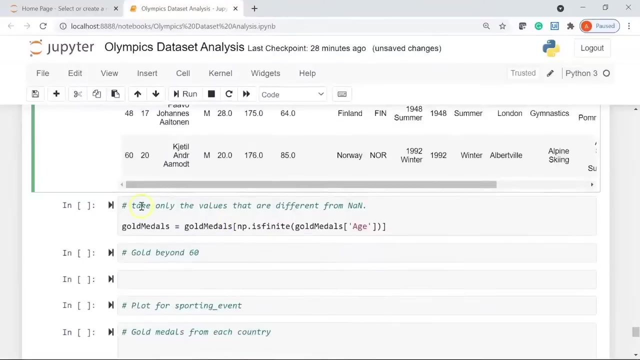 we have the top five rows of the athletes who have won a gold medal. you can see all the records have medal as gold. now we are going to use this subset of the data and perform some more analysis, so here i want to take only the values that are different from. 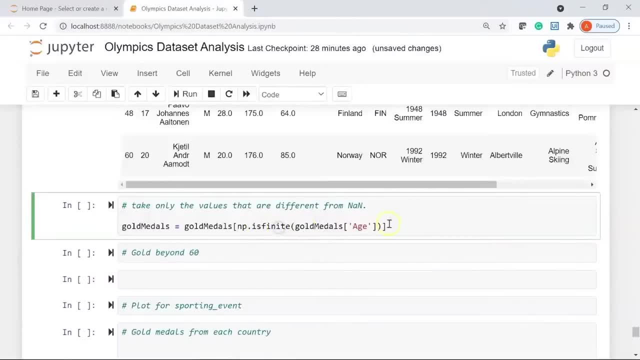 nan, so i am going to use is finite function and inside that i have said gold medals age. let me just run it cool now. i want to see the athletes who have secured a gold medal beyond the age of 60 years, which is very rare. so we will see. 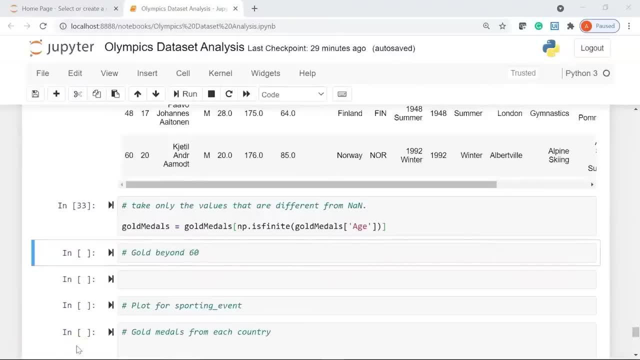 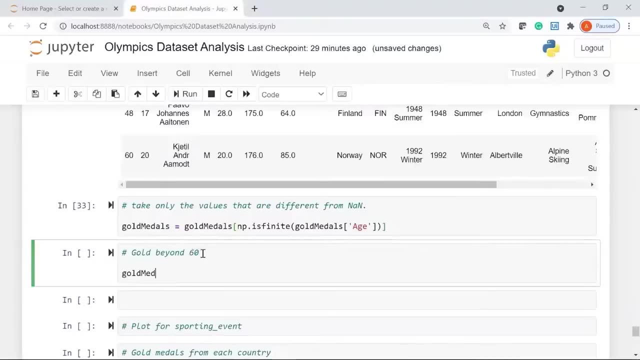 the total number of athletes with more than 60 years of age having won a gold medal. so here i am going to say gold medals, i will use my column as id and then i will use my variable gold medals and then i will say age should be. 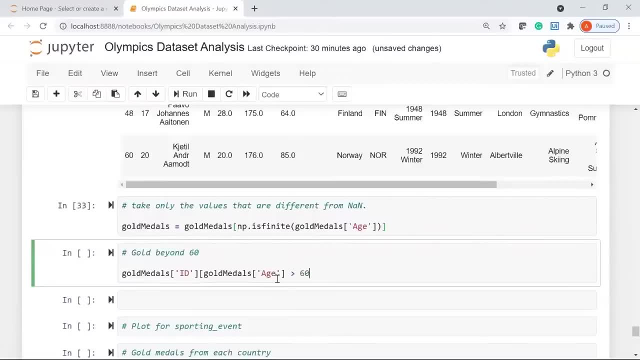 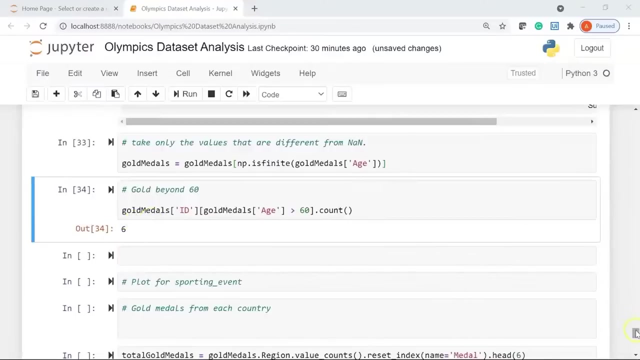 greater than 60 and then close my square bracket and say count. ok, let me just verify if everything is fine. yeah, i will run it and we will see the result. so there are total six athletes who have won a gold medal having age more than 60 years. 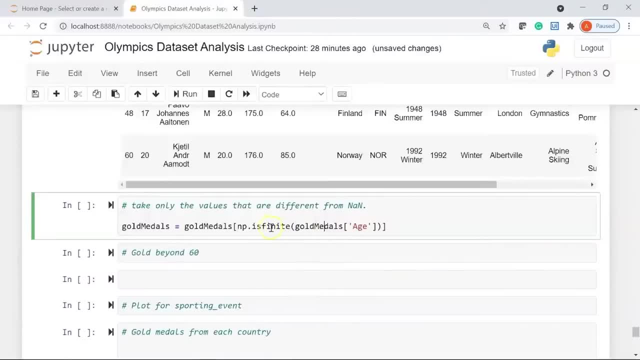 that are different from nan, so i am going to use is finite function and inside that i have said gold medals age. let me just run it cool now. i want to see the athletes who have secured a gold medal beyond the age of 60 years, which is very rare. 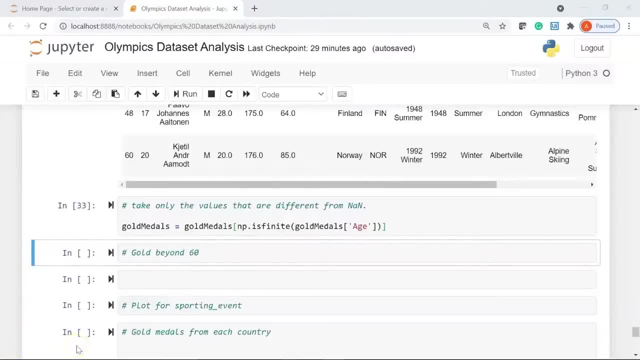 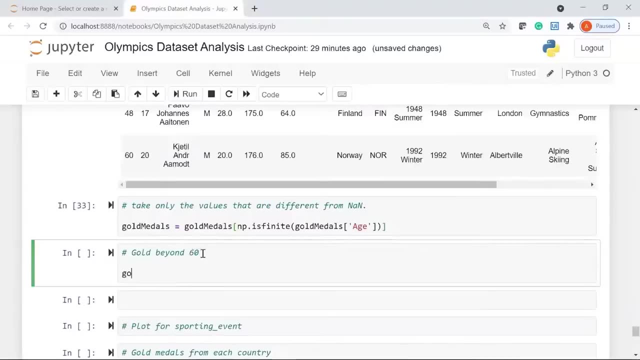 so we will see the total number of athletes with more than 60 years, of each having won a gold medal. so here i am going to say gold medals, i will use my column as id, and then i will use my variable gold medals, and then i will say: 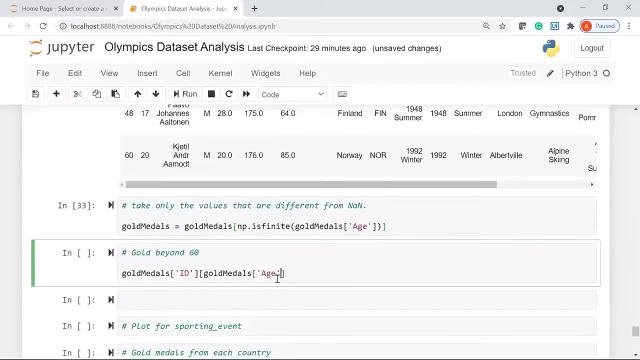 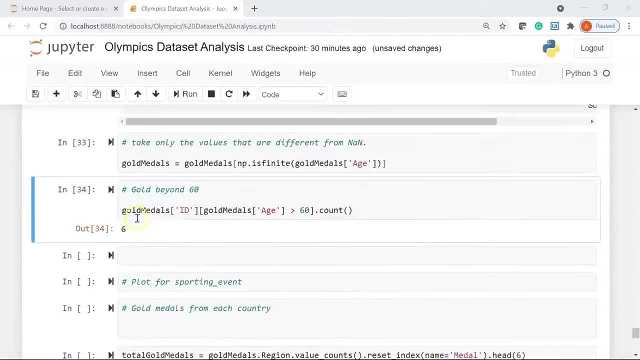 age should be greater than 60, and then close my square bracket and say count. ok, let me just verify. if everything is fine, yeah, i will run it and we will see the result. so there are total six athletes who have won a gold medal having age more than 60 years. 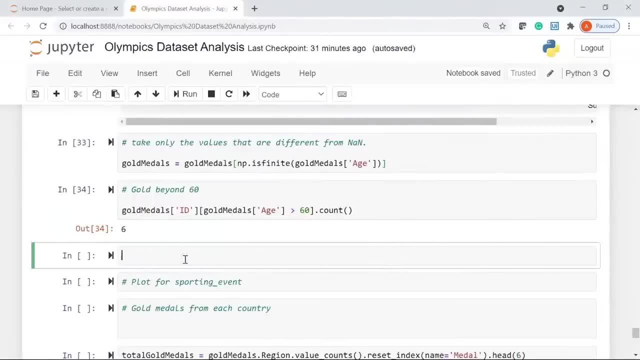 cool. now let me check for which sport these six gold medals have come. so i will say sporting underscore event. this is going to be my variable name. equal to, i will use the same variable name: gold medals. i will going to choose my sport column and then i will give. 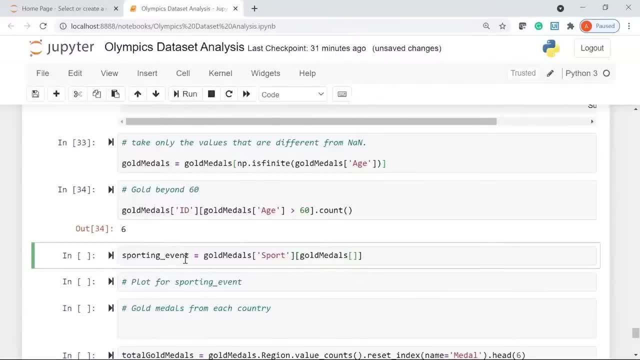 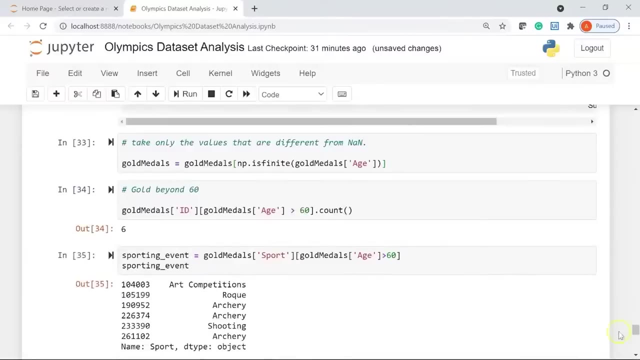 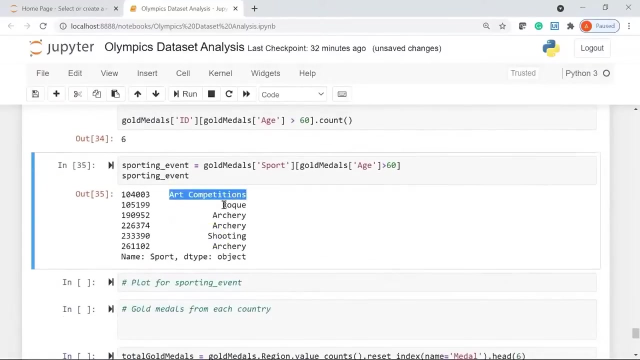 my condition: age greater than 60. now let's go ahead and we will print the variable sporting event. if i run this, you can see it here. so for art competitions, even for archery and shooting and this one called rook, we have had gold medals from: 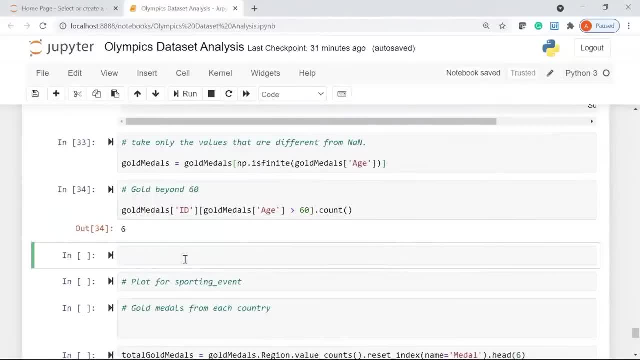 cool. now let me check for which sport these six gold medals have come. so i will say sporting underscore event. this is going to be my variable name. equal to, i will use the same variable name: gold medals. i will going to choose my sport column and then i will give. 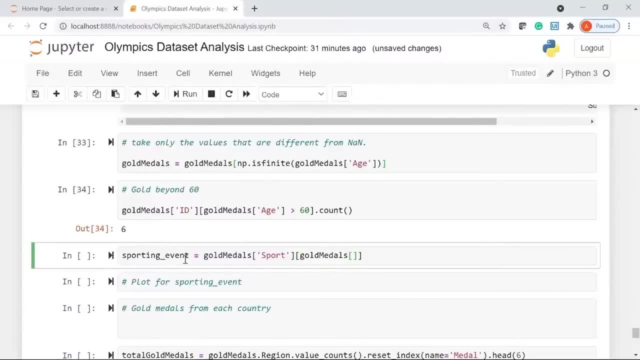 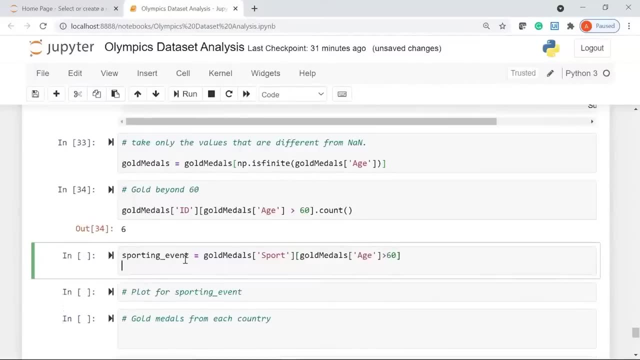 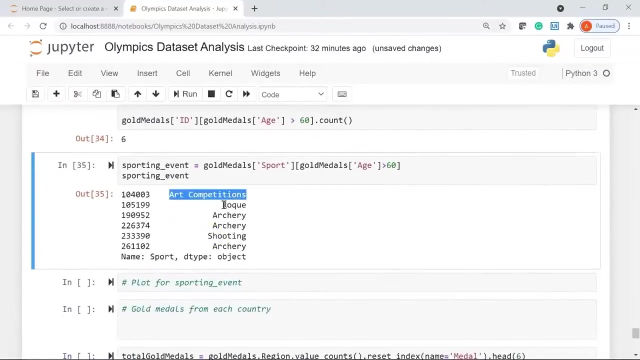 my condition: age greater than 60. now let's go ahead and we will print the variable sporting event. if i run this, you can see it here. so for art competitions, even for archery and shooting and this one called rook, we have had gold medals from athletes. 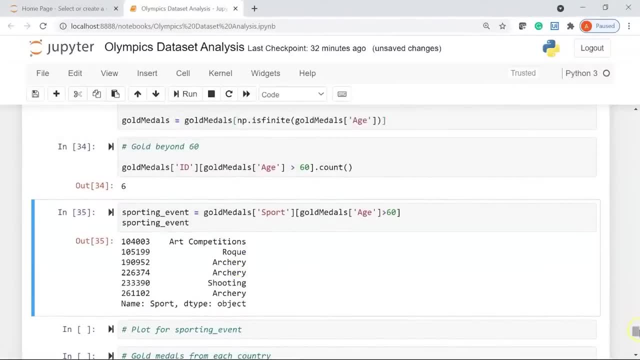 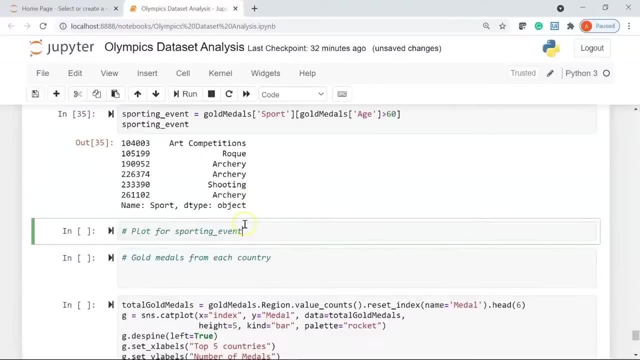 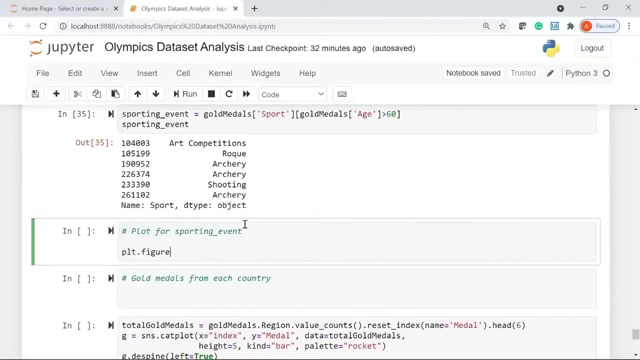 who had an age more than 60 years. now we are going to plot this result, or the table that we achieved, on the top. so i will say plt dot figure. i will give my figure size equal to, let's say, 10 comma 5. then i will say plt dot. 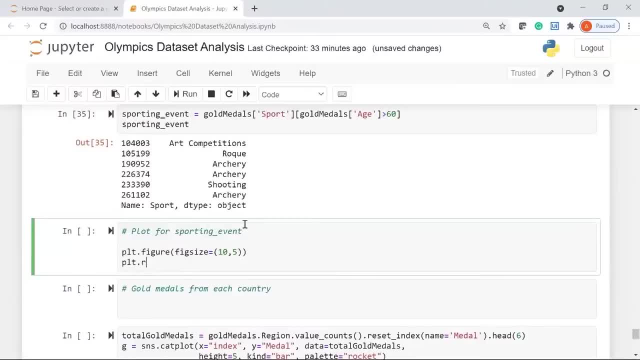 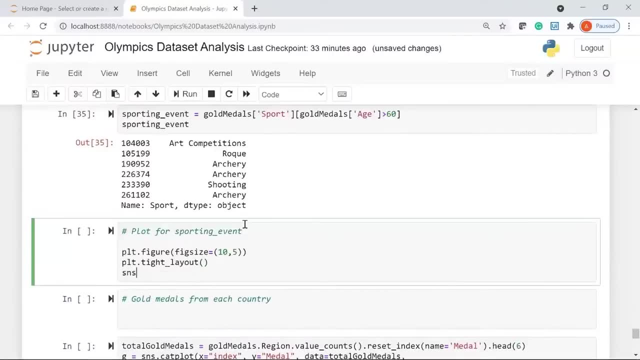 we will use the title tight layout: see tight underscore layout. then i am going to use the seaborn library and create a count plot for my variable sporting underscore event. then i will say plt dot title. i will give the title as gold medals for athletes over 60 years, of each. 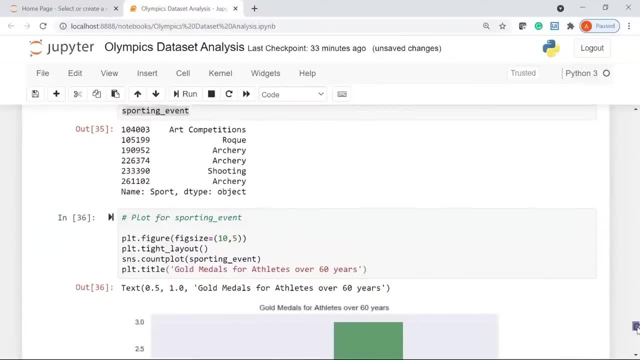 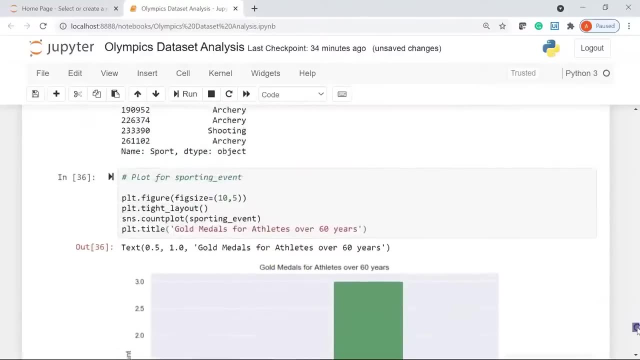 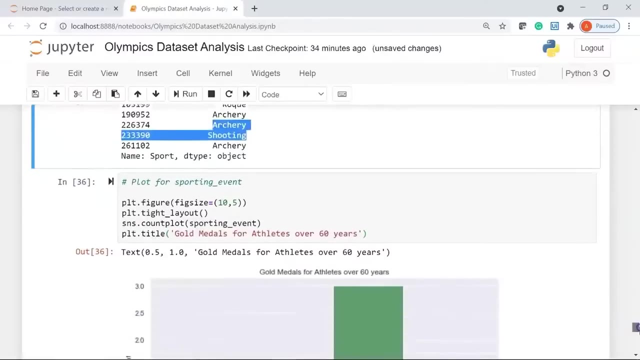 let's run it, and if i scroll down you can see here we have a nice count plot. i have my title, gold medals for athletes over 60 years and since for archery, we had 3 players who secured a gold medal having an age more than. 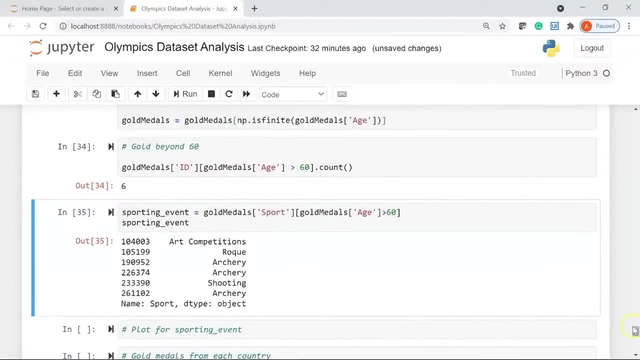 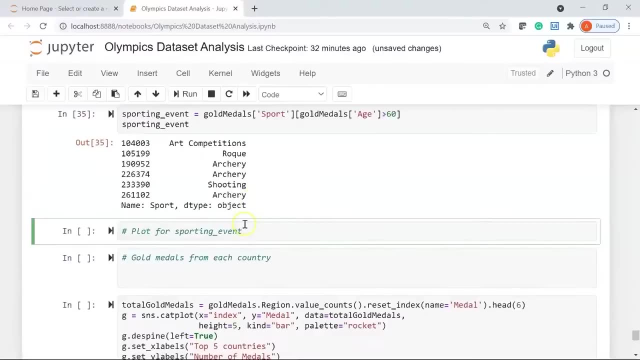 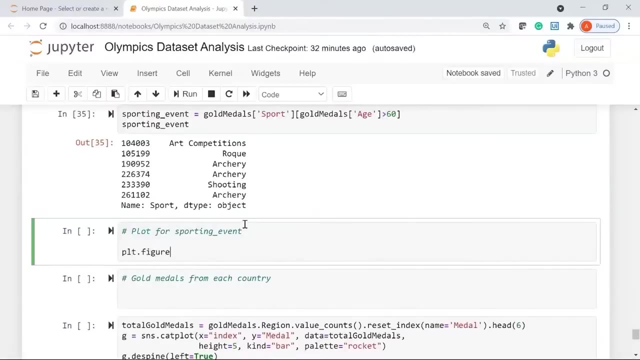 athletes who had an age more than 60 years. now we are going to plot this result, or the table that we achieved, on the top. so i will say plt, dot figure. i will give my figure size equal to, let's say, 10 comma 5. then 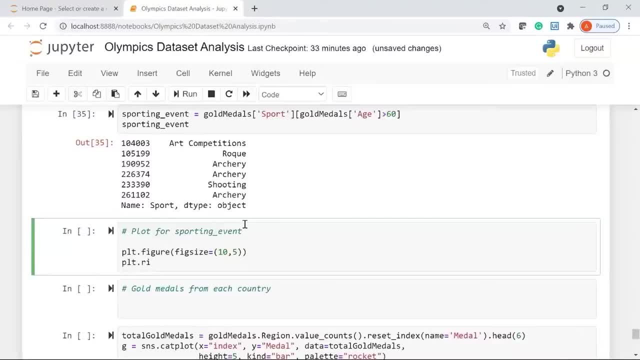 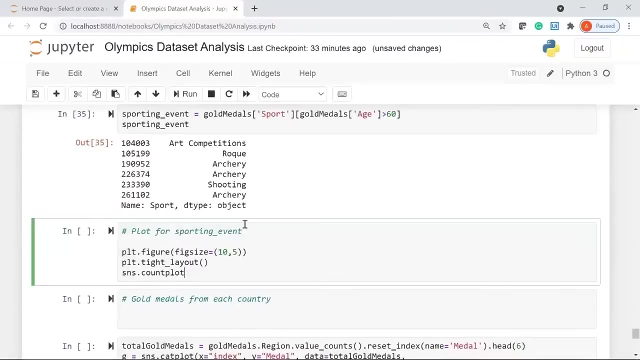 i will say plt dot. we will use the tight layout, say tight underscore layout. then i am going to use the seaborn library and create a count plot for my variable sporting underscore event. then i will say plt dot. title. i will give the title as gold medals for athletes. 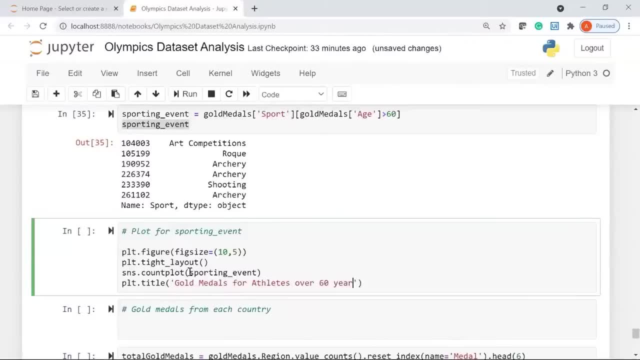 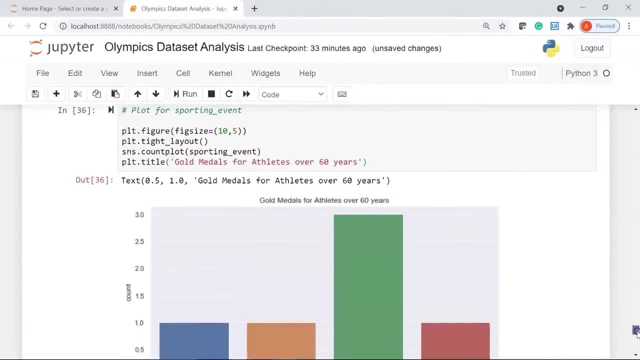 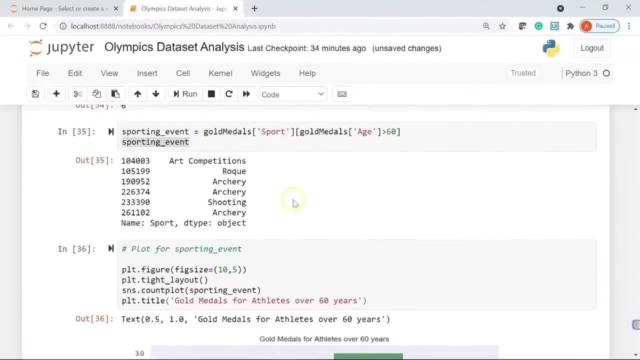 over 60 years of age. let's run it, and if i scroll down you can see here we have a nice count plot. i have my title- gold medals for athletes over 60 years, and since for archery we had 3 players who secured a gold medal, 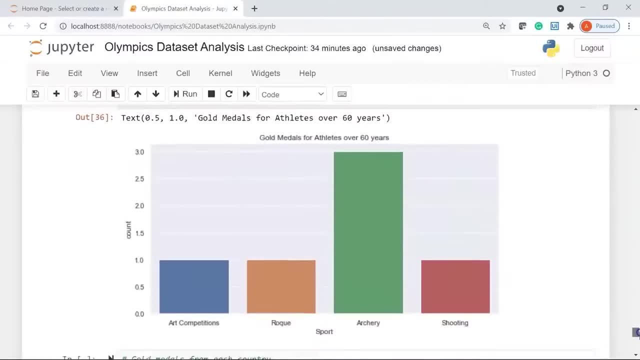 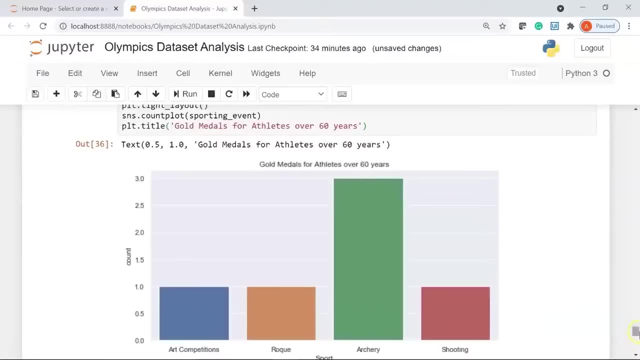 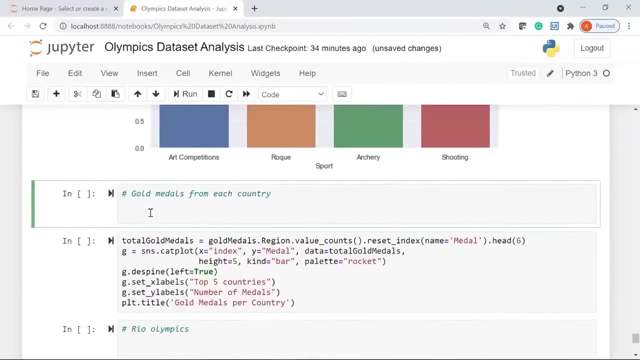 having an age more than 60 years. you can see here: archery is 3, art competition 1, rook is 1 and shooting. we had 1 medal. alright, now we will see the total gold medals from each country. so for that i will say: 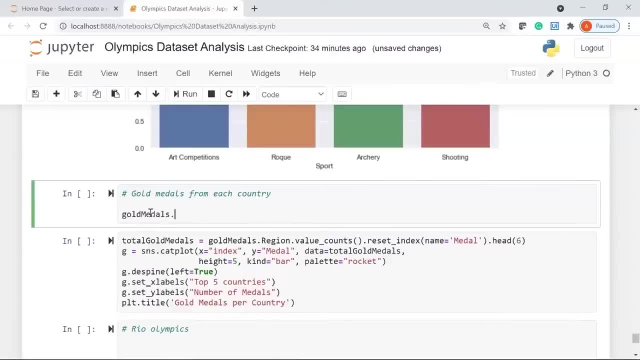 gold medals dot. we will use the region column and followed by that, i will use the value underscore counts function and i will reset the index with name equal to. i will provide the medal column. then we are going to print the head for the top 5 countries. let me 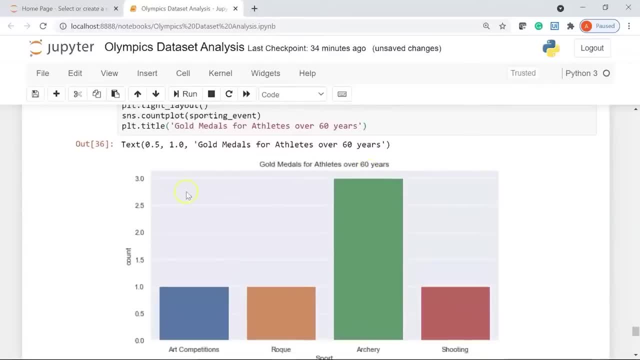 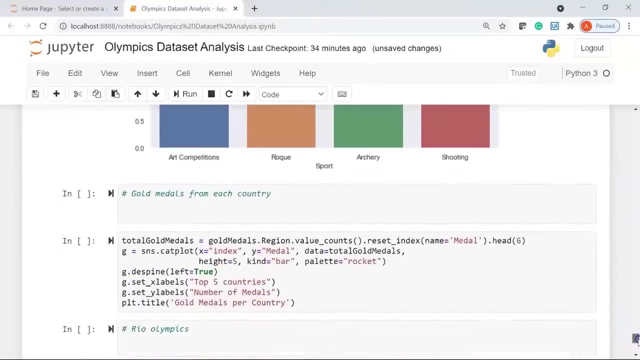 60 years. you can see here: archery is 3, art competition 1, rook is 1 and shooting we had 1 medal. alright, now we will see the total gold medals from each country. so for that i will say gold medals dot. we will use the 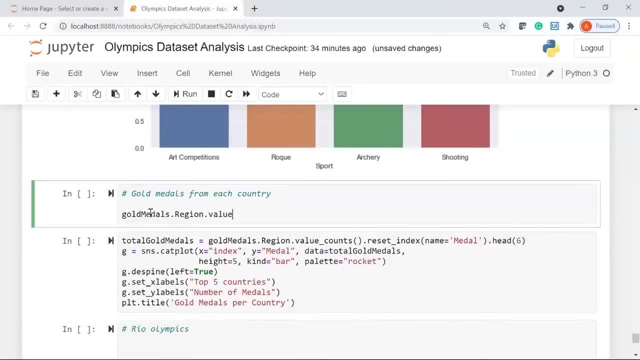 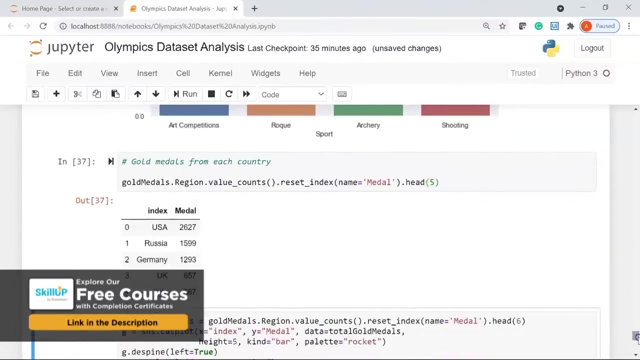 region column and followed by that, i will use the value underscore counts function and i will reset the index with name equal to. i will provide the medal column. then we are going to print the head for the top 5 countries. let me run it. you can see it here. 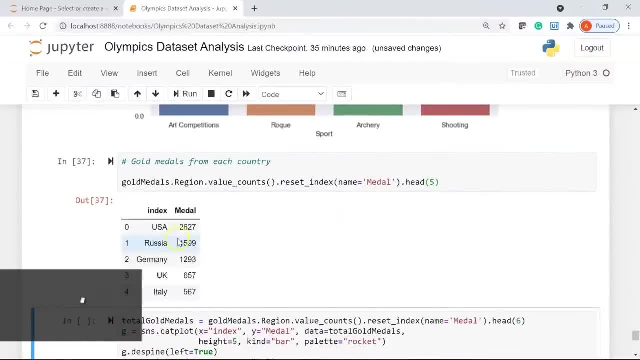 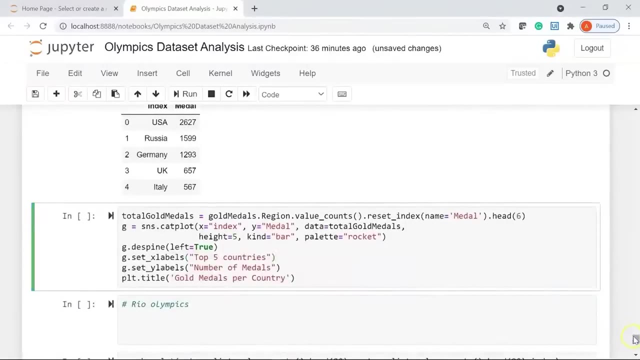 so USA has secured the most number of gold medals. then we have Russia, Germany, UK and then we have Italy. cool. now in this cell, i am going to create a plot to visualize the table that i got above. so i have used my labels, my titles, i am using the cat plot function. 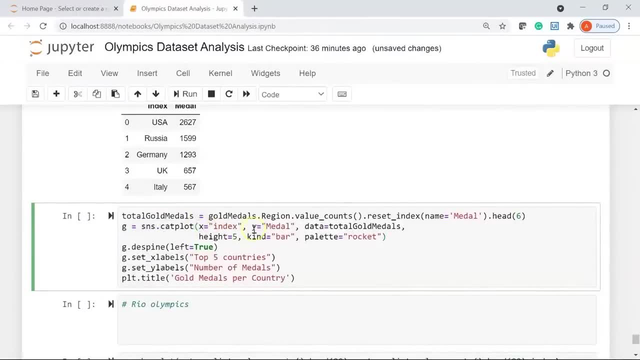 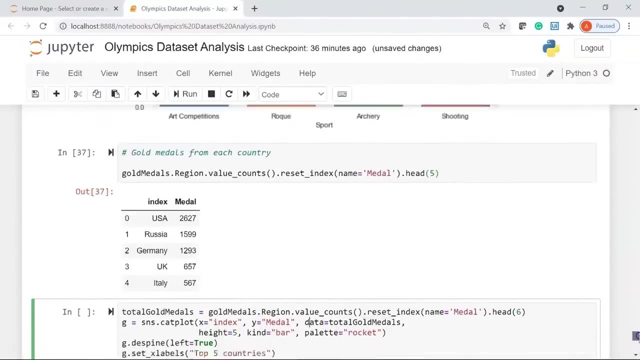 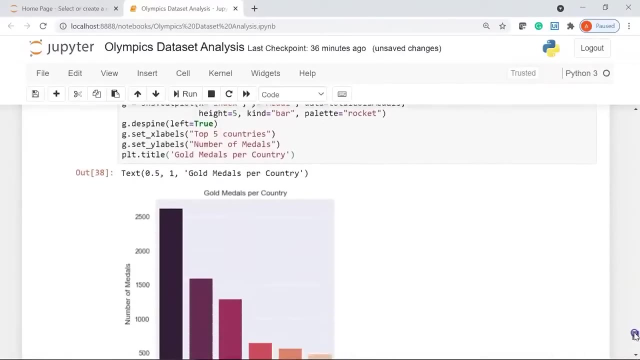 that is present in the seaborn library. i have my x-axis, my y-axis, the data which is total gold medals. let me just verify, ok, and we will run it. if i scroll down, you can see this is a different palette that i had used, which is rocket. 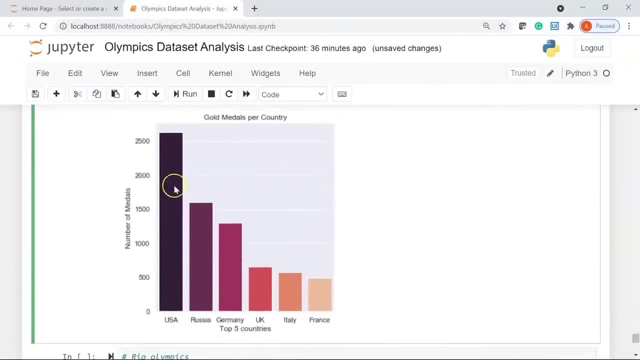 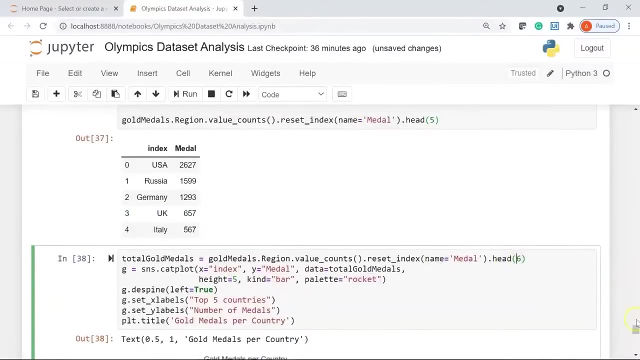 and you can see USA has got the most number of gold medals. then we have Russia, Germany, UK, Italy and France. now we also have included France here, which was not present in this table, the reason being i have used head as 6, so it will give me. 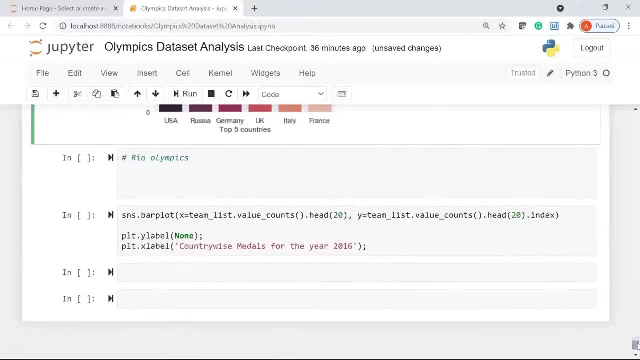 the top 6 countries. alright, now we will analyze and look at the data for the most recent Olympic event that is present in our data set. i am talking about the 2016 Rio Summer Olympics. so, first of all, i will create a variable called max year. 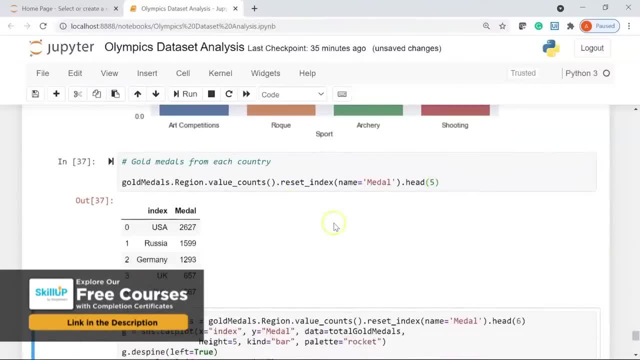 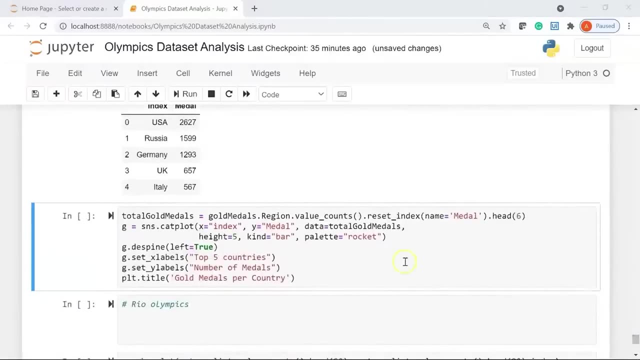 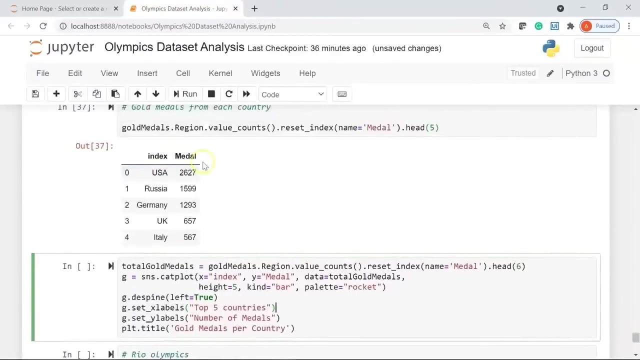 run it. you can see it here. so USA has secured the most number of gold medals. then we have Russia, Germany, UK and then we have Italy. cool. now in this cell i am going to create a plot to visualize the table that i got above. so i have used my labels, my 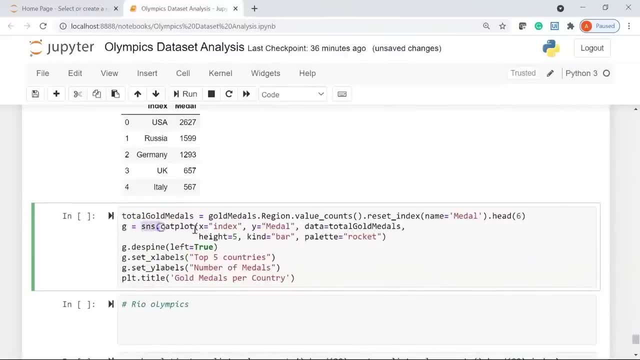 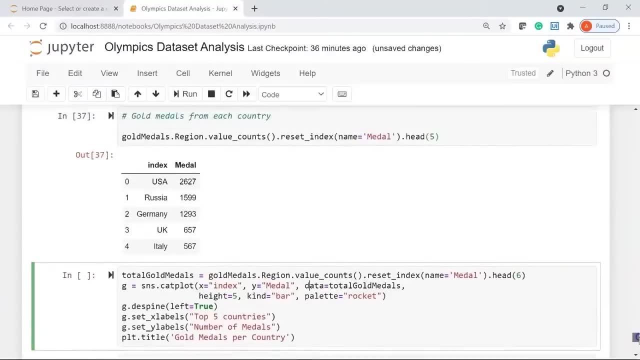 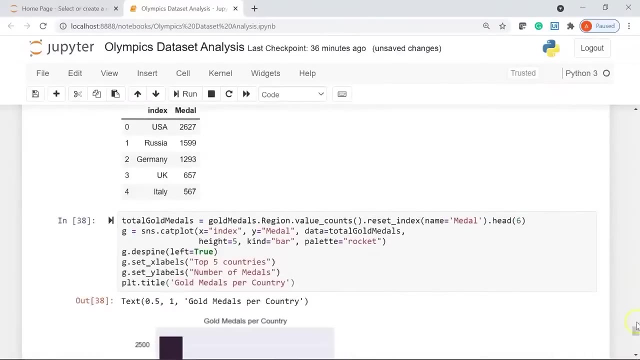 titles. i am using the cat plot function that is present in the seaborn library. i have my x axis, my y axis, the data which is total gold medals. let me just verify, ok, and we will run it. if i scroll down, you can see this is a different palette that i had used. 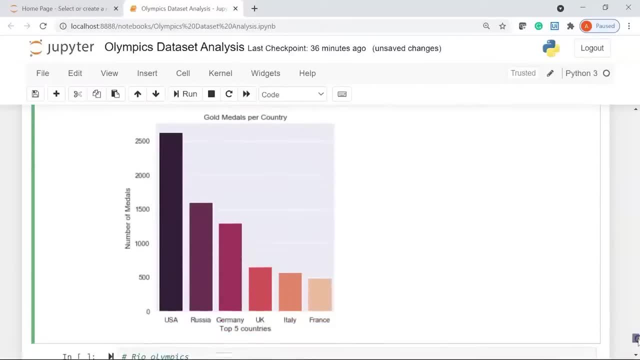 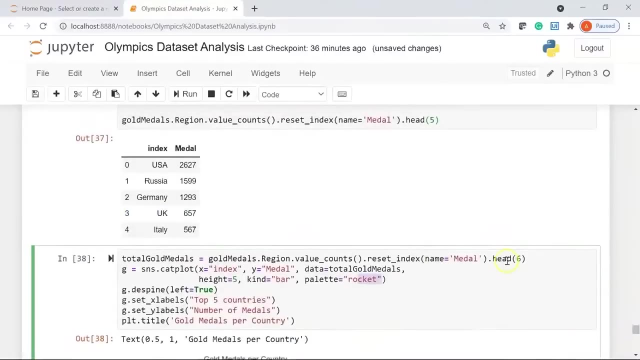 which is rocket, and you can see USA has got the most number of gold medals. then we have Russia, Germany, UK, Italy and France. now we also have included France here, which was not present in this table, the reason being i have used head as 6, so we will get. 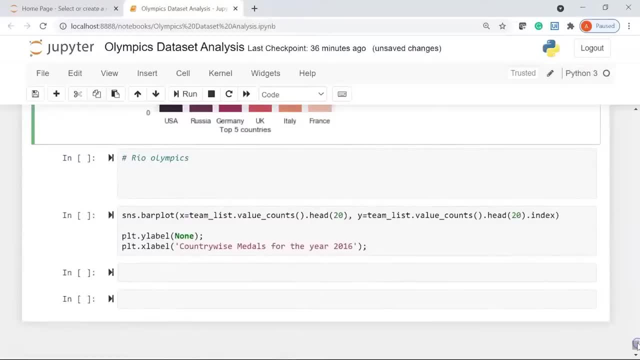 the top 6 countries. alright, now we will analyze and look at the data for the most recent Olympic event that is present in our data set. i am talking about the 2016 Rio Summer Olympics. so, first of all, i will create a variable called max year. 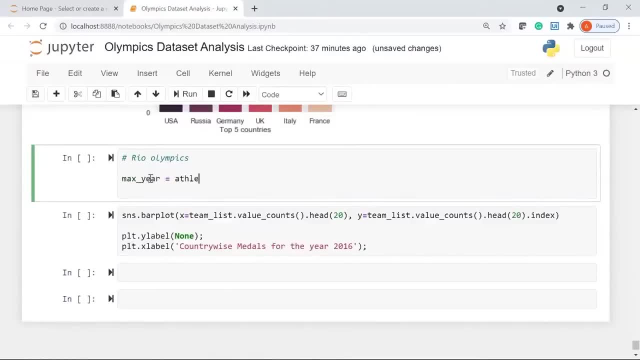 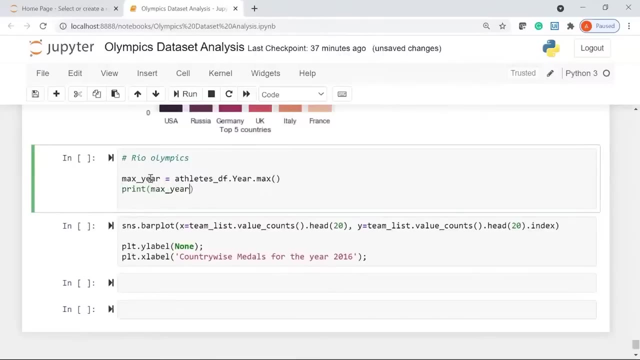 which will be equal to my data frame name athletes. underscore df, my column name, year, and i will use the max function. then let's go ahead and print my max year. i will just show you the output you can see here. my max year present in the data set is: 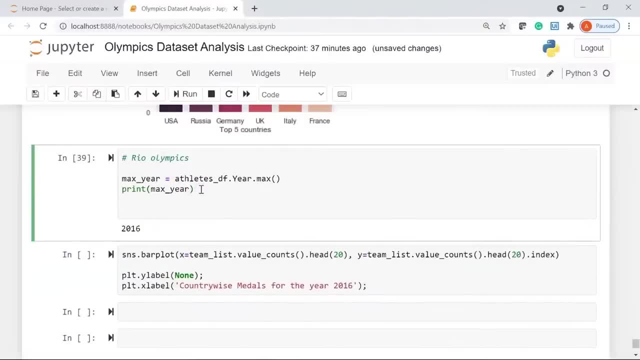 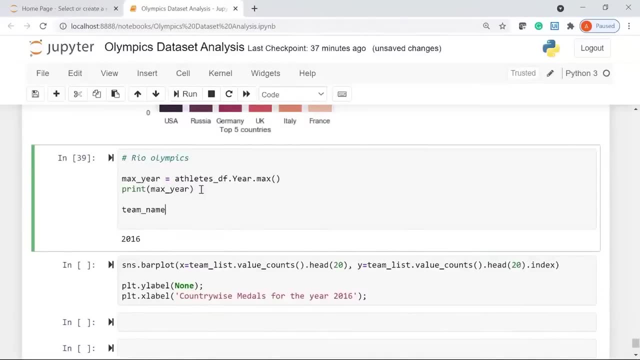 2016: the Rio Olympics. next, we will create another variable called team underscore names. that will be equal to my data frame name. athletes underscore df- within square brackets i will give parenthesis and then say: athletes underscore df. dot year should be equal to equal to my output. that is max year. 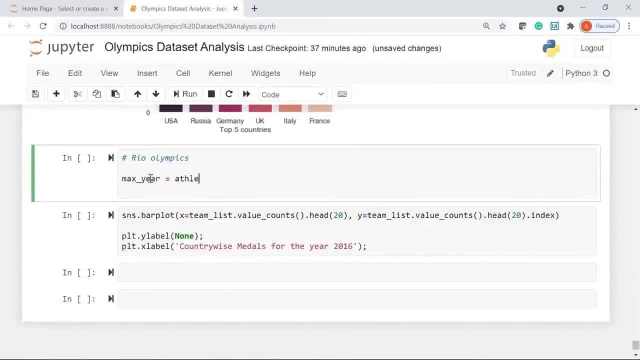 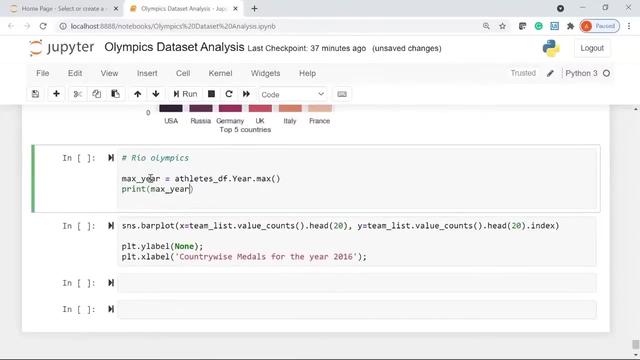 which will be equal to my data frame name athletes. underscore df, my column name, year, and i will use the max function. then let's go ahead and print my max year. i will just show you the output you can see here. my max year present in the data set is: 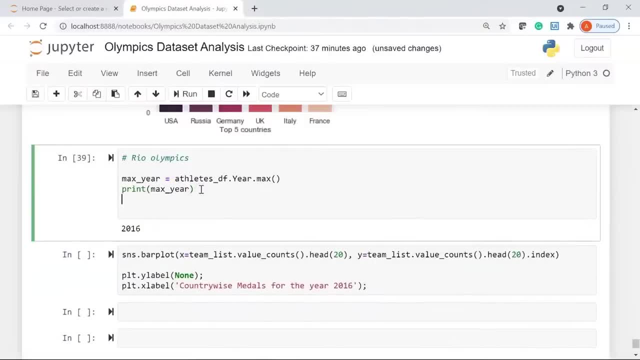 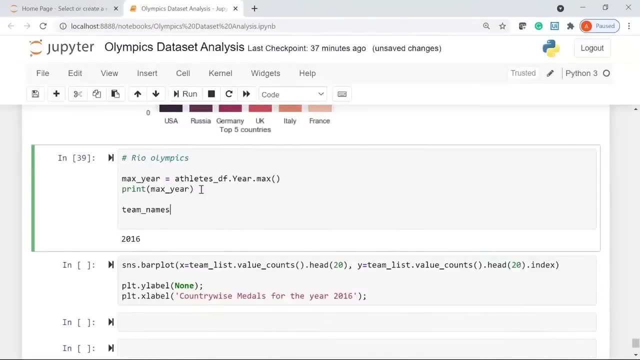 2016: the Rio Olympics. next, we will create another variable called team underscore names. that will be equal to my data frame name. athletes underscore df- within square brackets i will give parenthesis and then say: athletes underscore df. dot year should be equal to equal to my output. that is max year. 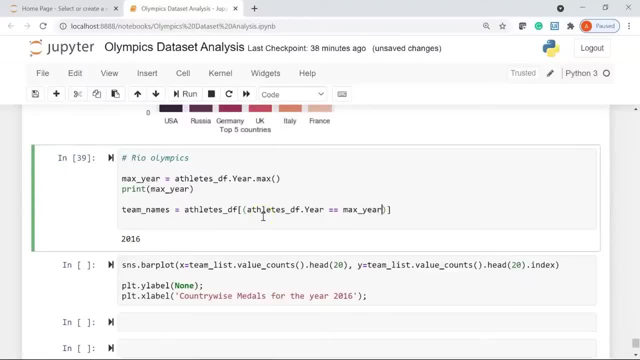 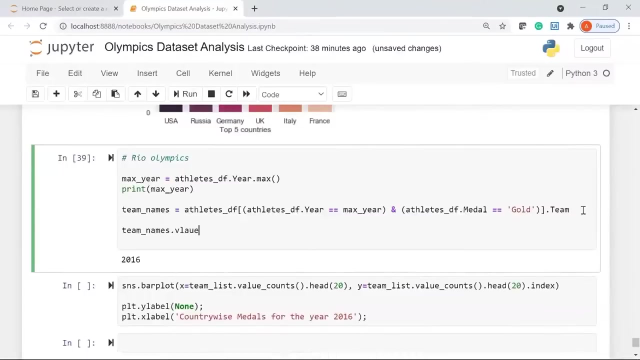 which is actually 2016. then i will say ampersand. i will just copy this, paste it here. this time i will use the middle column and say equal to equal to gold. i will say dot team and then i will say team underscore names: dot value. 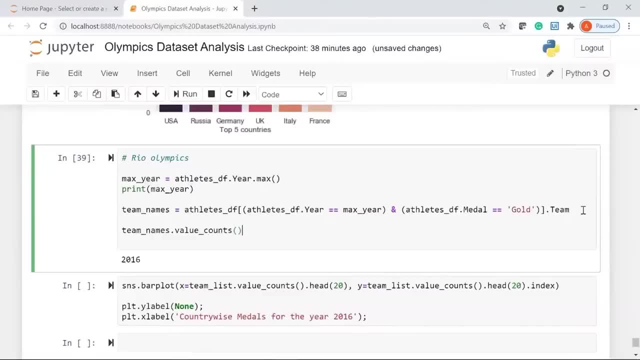 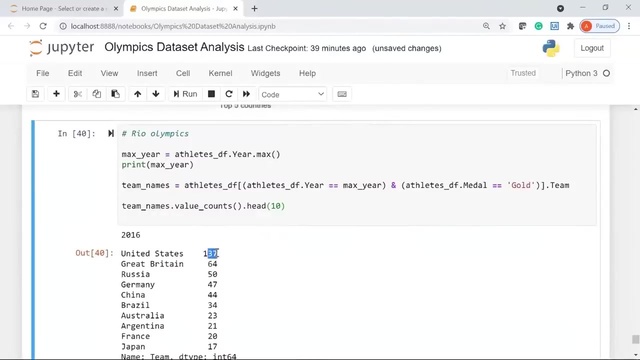 underscore counts dot head and will display the top 10 countries. let me run this. there you go. so in Rio Olympics, United States secured the most number of gold medals. now, the reason this is 137 is we have also counted the team events, for example basketball. similarly, Great Britain had 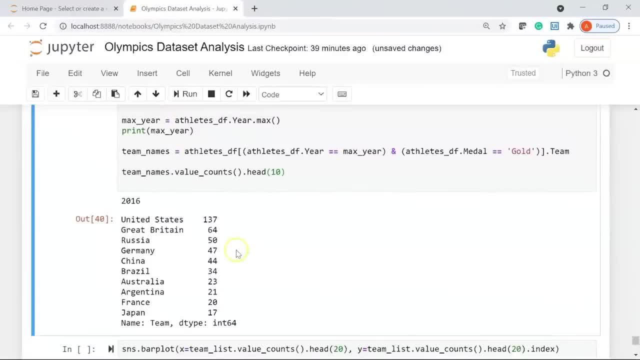 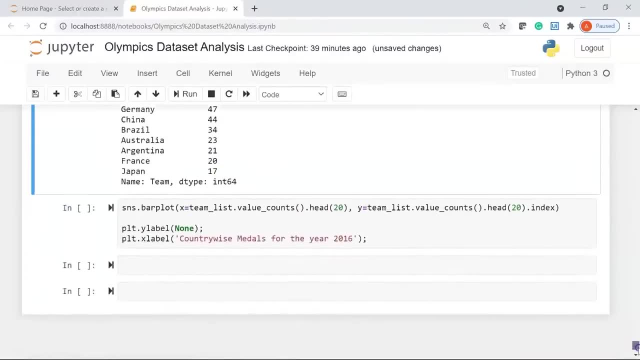 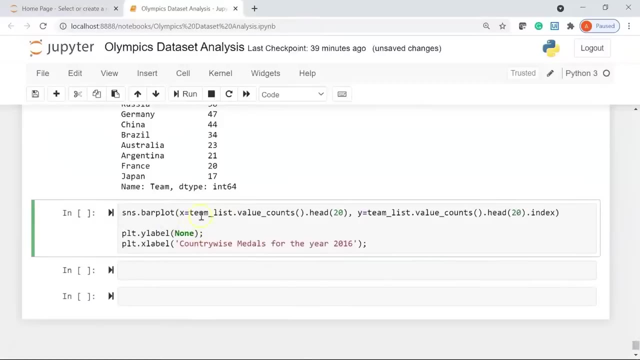 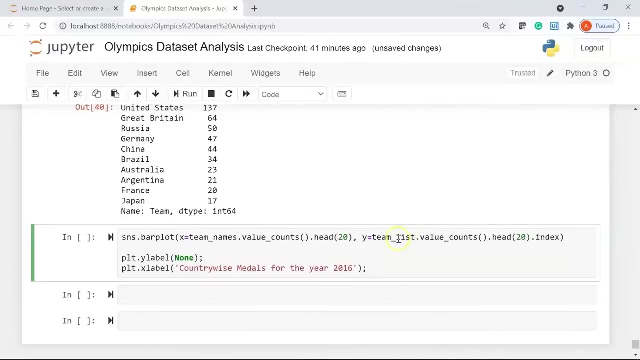 64 gold medals in total, Russia 50, we have Brazil 34, Argentina 21, France 20 and Japan 17. alright, now, using the above result, we are going to create a bar plot. i will just change this team underscore list to team underscore names. similarly, here also, i will make the 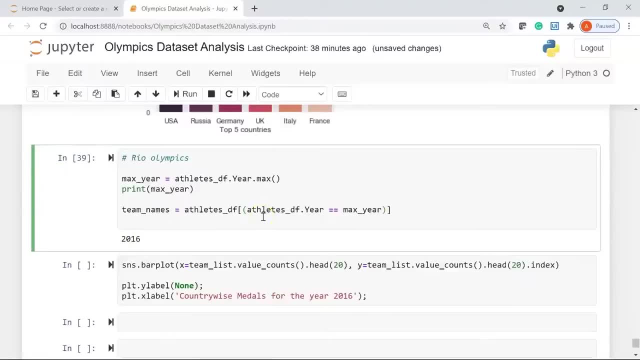 which is actually 2016. then i will say ampersand. i will just copy this, i will paste it here. this time i will use the middle column and say equal to equal to gold. i will say dot team. then i will say team underscore names: dot team. 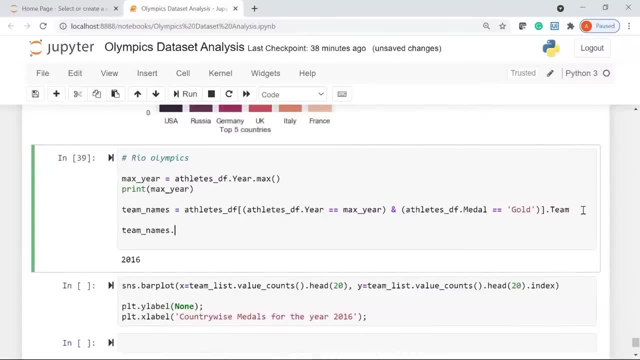 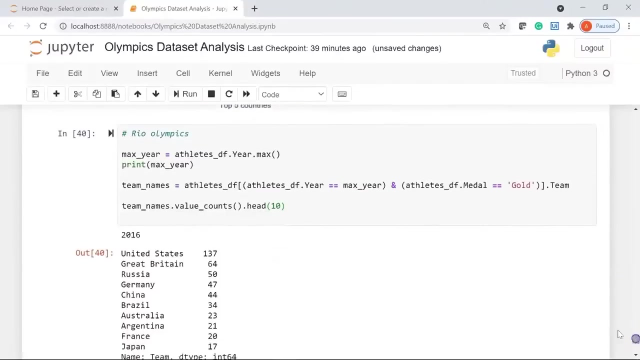 then i will say team underscore, dot value, underscore counts, dot head and will display the top 10 countries. let me run this. there you go. so in Rio Olympics, United States secured the most number of gold medals. now, the reason this is 137 is we have also 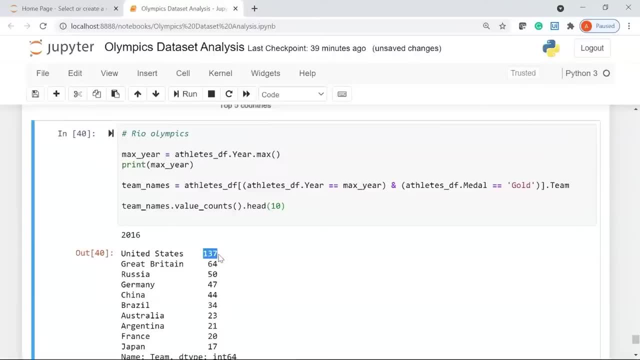 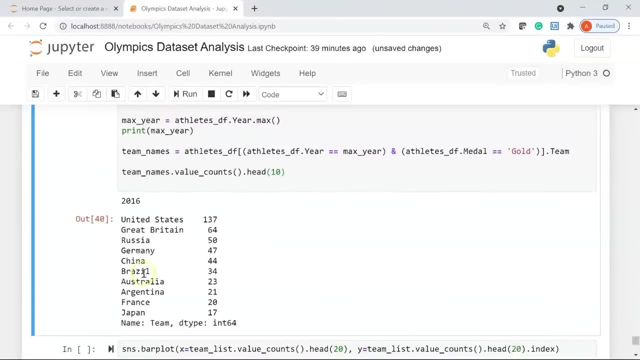 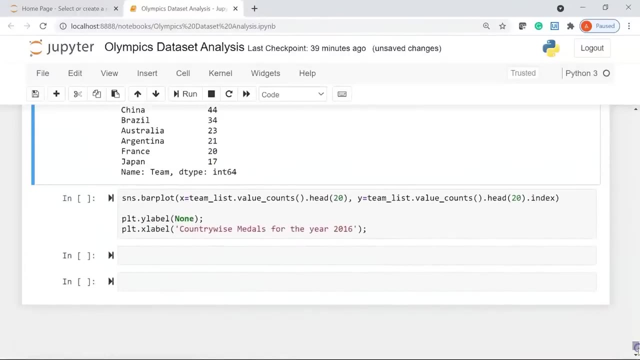 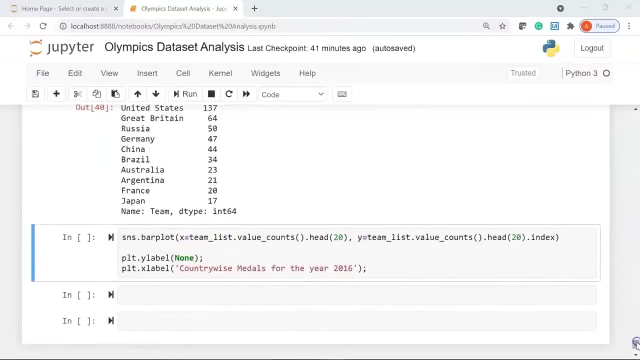 counted the team events, for example basketball. similarly, Great Britain had 64 gold medals in total, Russia 50, we have Brazil 34, Argentina 21, France 20 and Japan 17. alright, now, using the above result, we are going to create a bar plot. i will just change. 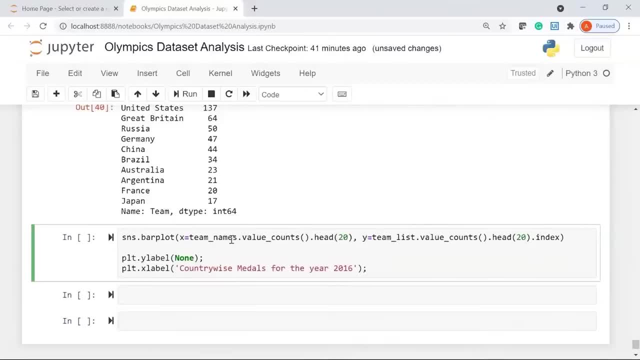 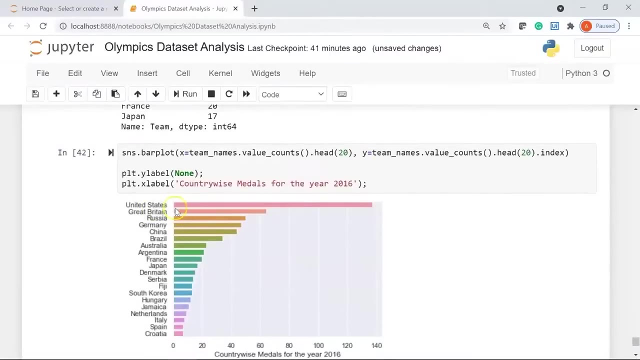 this team underscore list to team underscore names. similarly, here also i will make the corrections as team underscore names. cool, now we will run it and you can see here we have a nice horizontal bar plot. so we have United States at the top: Great Britain, Russia, Germany, China, Brazil. 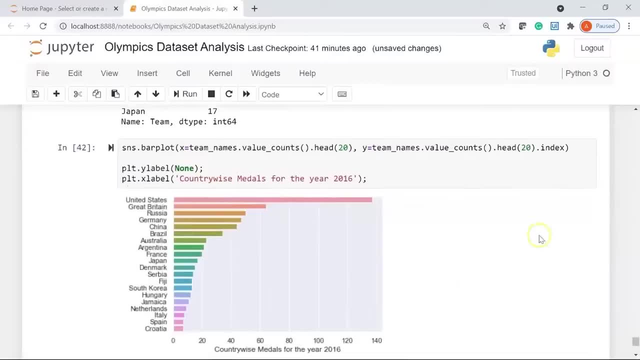 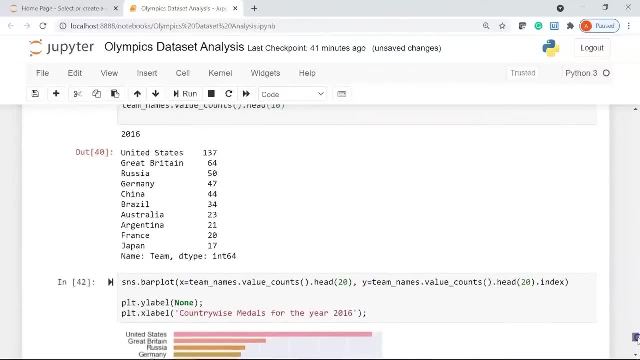 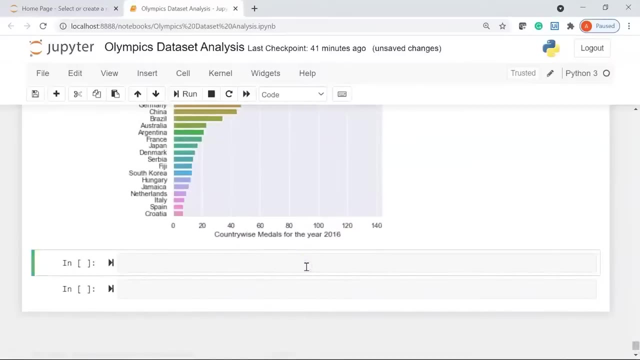 so here i am displaying the top 20 nations, since i have used head as 20, so these are the top 20 nations who secured the most number of gold medals in the Rio Olympics. alright, now, in the final section of this video, we will create a scatter plot to visualize the 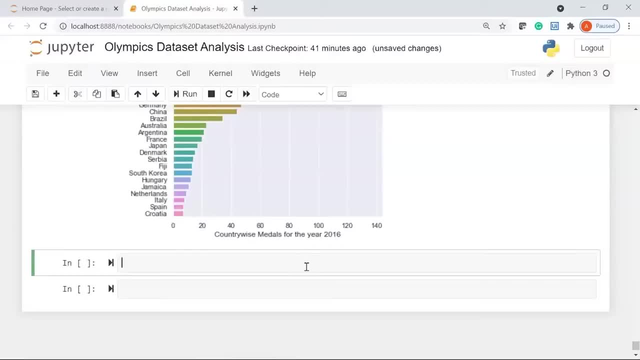 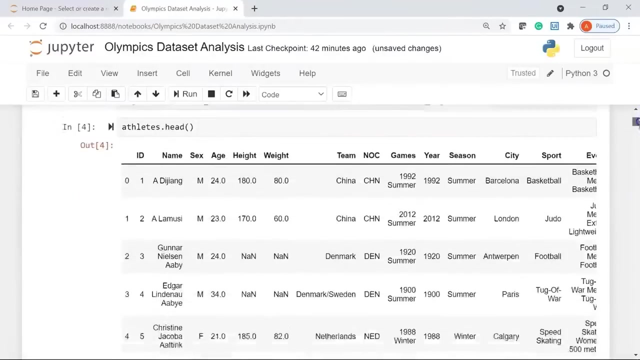 height and weight of male and female athletes who have won a medal now. it can be a gold medal, a silver medal or a bronze medal, but before that we need to filter the data only for athletes who have won a medal now. if you had noticed here our 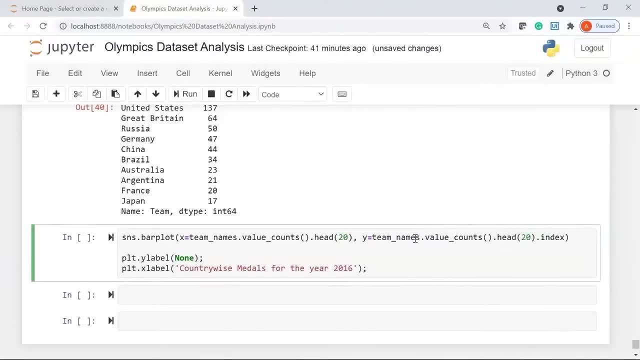 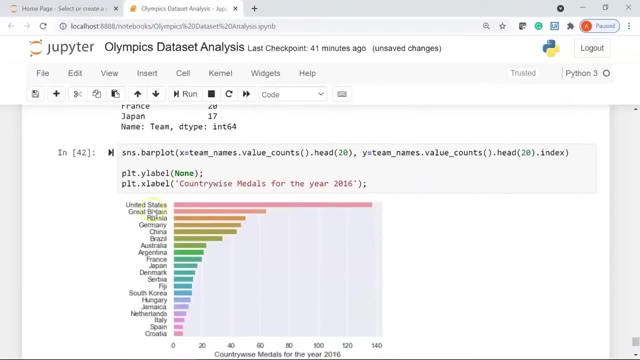 corrections as team underscore names. cool, now we will run it and you can see here we have a nice horizontal bar plot. so we have United States at the top: Great Britain, Russia, Germany, China, Brazil. so here i am displaying the top 20 nations, since i have used head as 20. 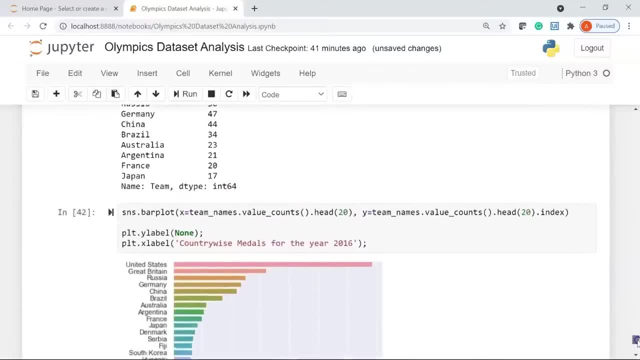 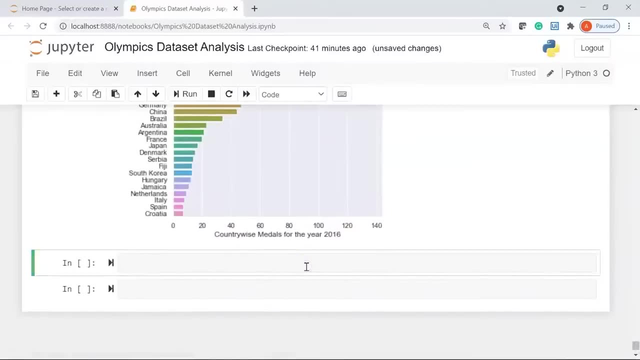 so these are the top 20 nations who secured the most number of gold medals in the Rio Olympics. alright, now, in the final section of this video, we will create a scatter plot to visualize the height and weight of male and female athletes who have won a medal. 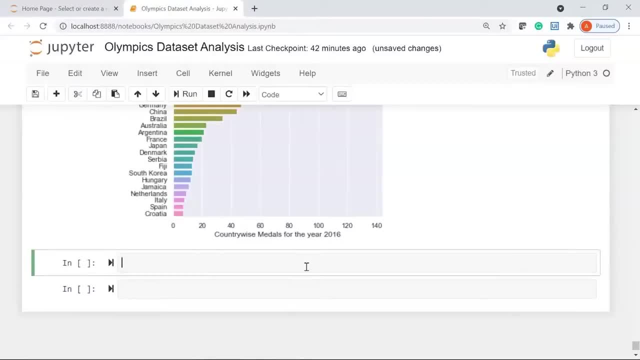 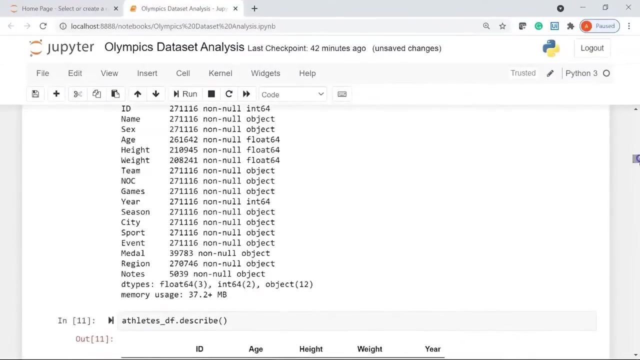 now it can be a gold medal, a silver medal or a bronze medal, but before that we need to filter the data only for athletes who have won a medal. now, if you had noticed, here our medals column also had a few null values, so we are not going to. 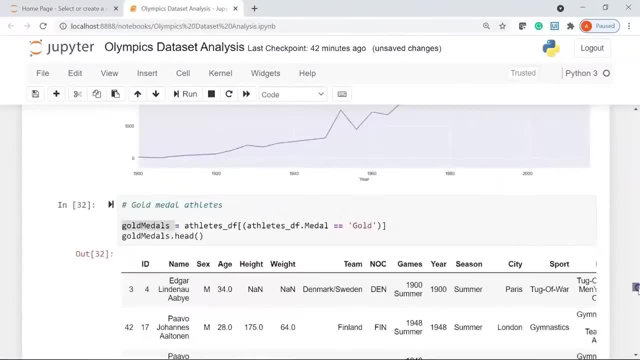 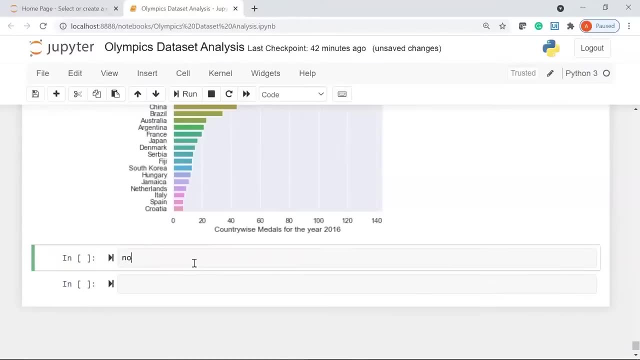 consider those null values. here we are only going to consider for the athletes who have won a medal. so for that i will create a variable called not underscore, null, underscore. medals equal to, i will say, athletes underscore df, then i will give my, lets make it df, i will give my condition. 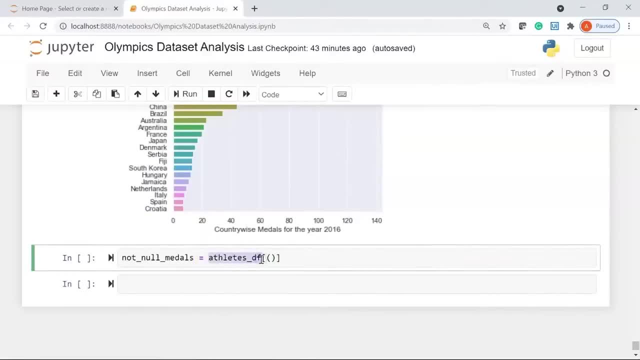 let me just copy this. i will paste it here, and then i will give my condition height and use the not null function and then i will say ampersand. create another parenthesis. i will say athletes underscore df. this time we will consider the weight column. again, i will use the function. 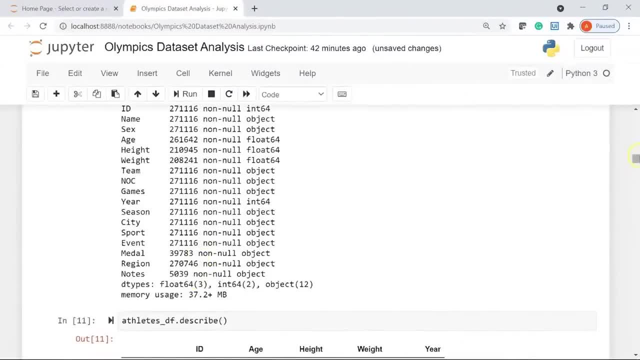 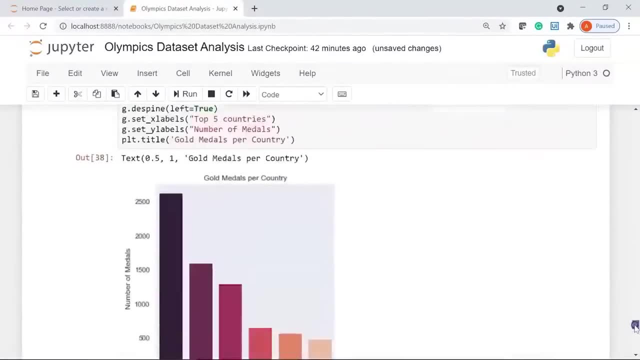 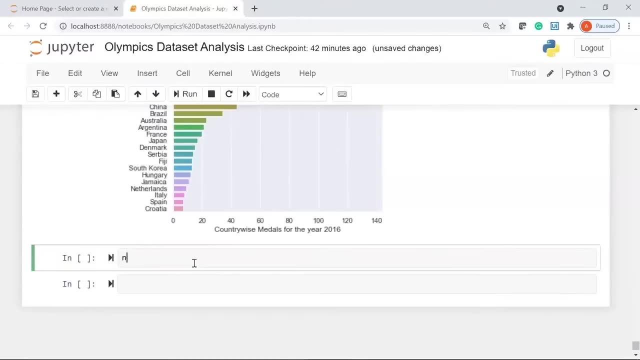 medals column also had a few null values. so we are not going to consider those null values here. we are only going to consider for the athletes who have won a medal. so for that i will create a variable called not underscore- null, underscore medals equal to. i will say: 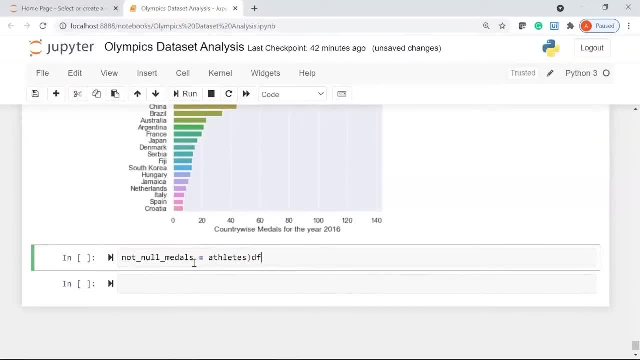 athletes underscore df, then i will give my let's make it df. i will give my condition. let me just copy this: i will paste it here and then i will paste it here, and then i will paste it here and then i will give my condition: height and use. 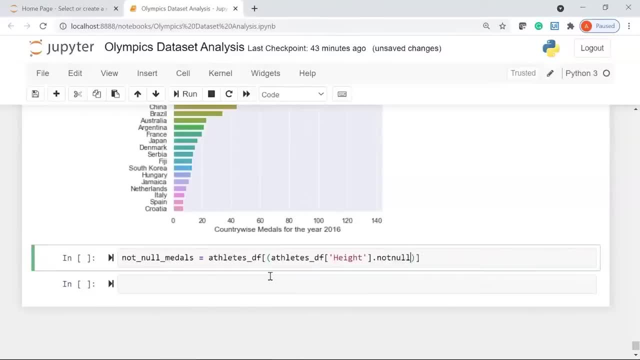 the not null function and then i will say ampersand. create another parenthesis. i will say athletes underscore df. this time we will consider the weight column again, i will use the function as not null and i will close the parenthesis. ok, i had missed one s here, cool. 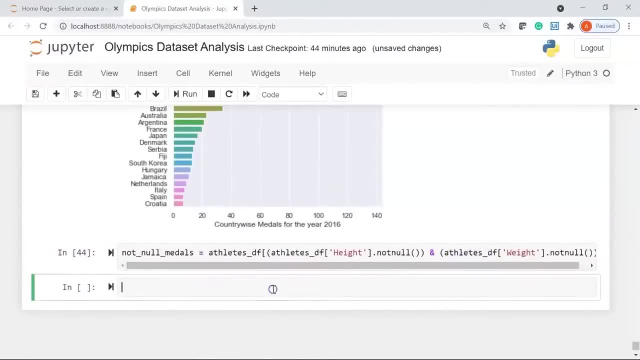 let me just run it now. alright, now we are going to create our final plot. i will say plt, dot figure. i will give my figure size equal to. i will say 12 comma 10. i will say axis equal to sns dot. we will be creating a scatter plot to plot. 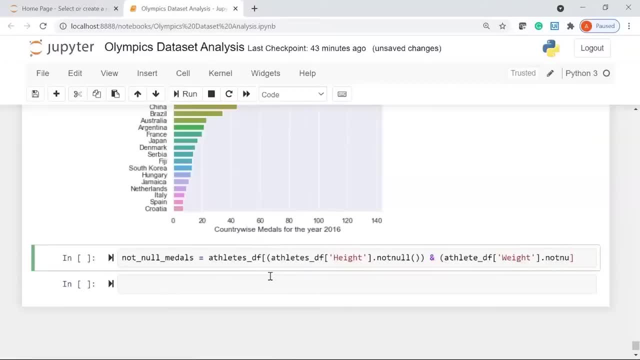 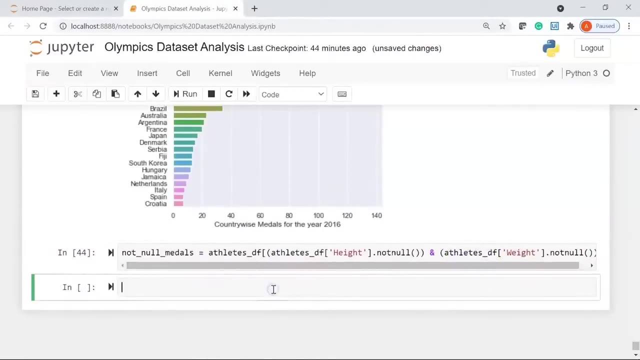 as not null, and i will close the parenthesis. okay, i had missed one s here. cool, let me just run it now. alright, now we are going to create our final plot. i will say plt dot figure. i will give my figure size. i will give my figure size. 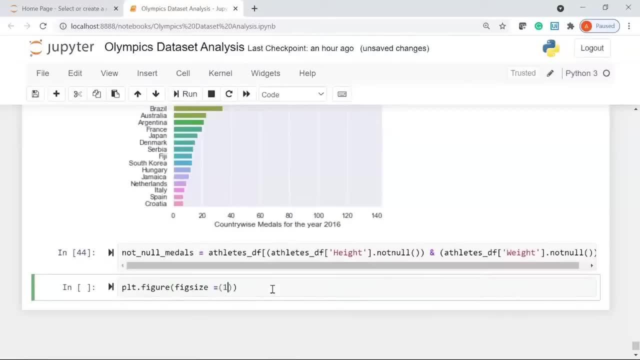 equal to. i will say twelve comma ten. i will say axis equal to axis equal to sns dot. we will be creating a scatter plot to plot the weight of the athletes who have won a medal. i will say scatter plot. in my x axis i will have height. 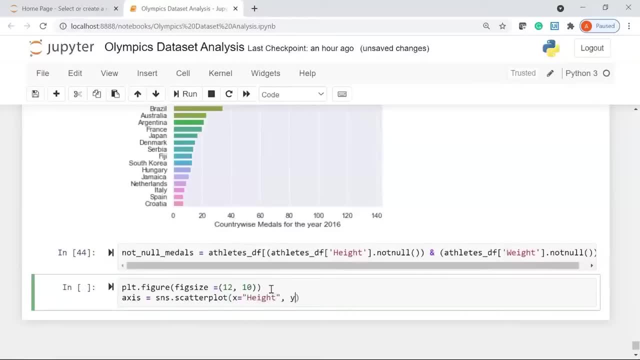 comma. in my y axis i will have weight comma. my data should be not underscore null, underscore medals. so this is what we created here: not underscore null, underscore medals comma. i will use hue equal to my sex column, cool. finally, i will say plt dot. i will give a title to my plot. 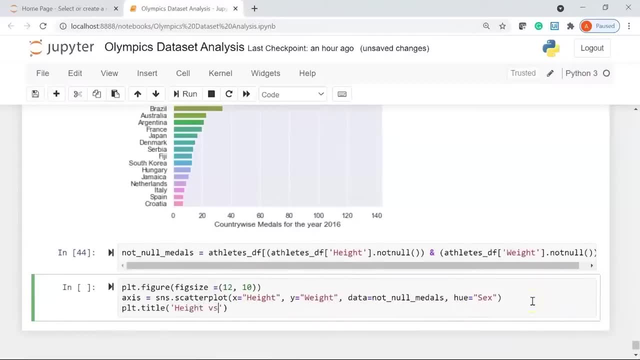 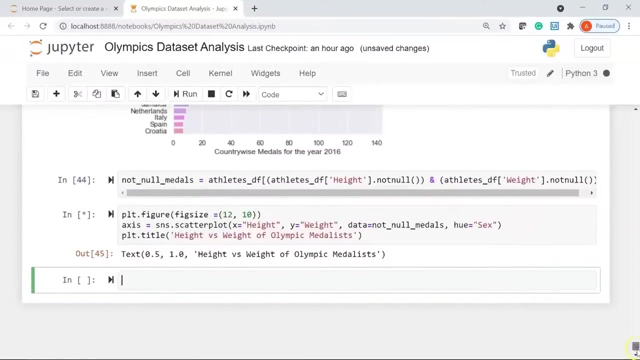 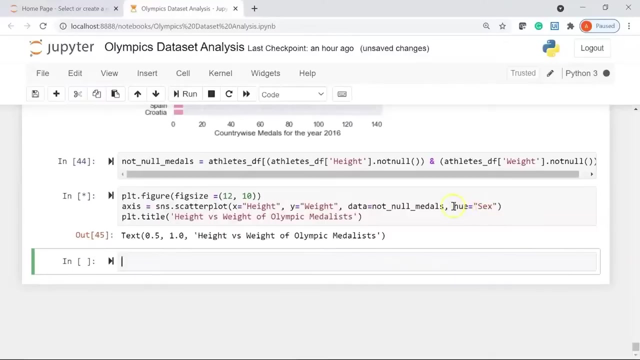 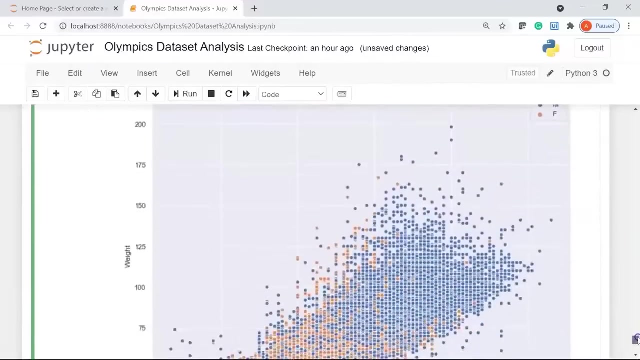 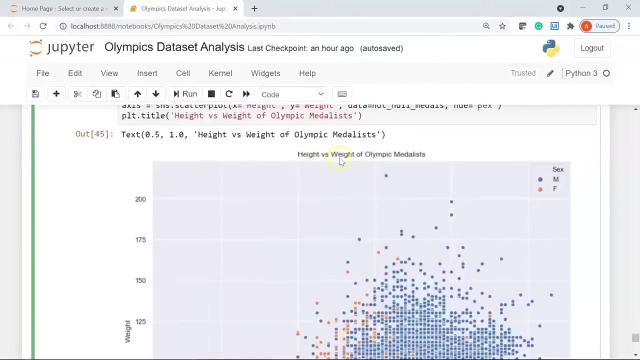 saying height versus weight of olympics, olympics being wearing muscles. how mustache of olympics is fit of of down. you can see here we have a nice scatter plot. on the top you have the title of the plot saying height versus weight of Olympic medalists. you can see. 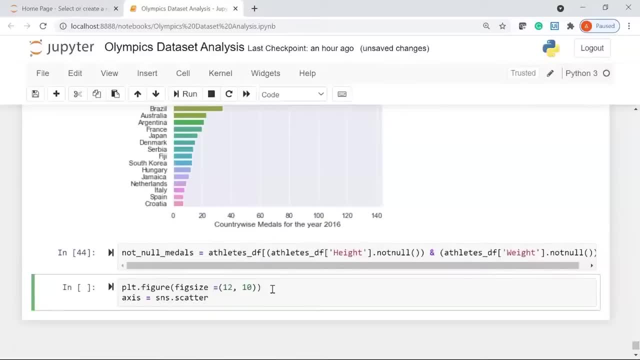 the height and weight of the athletes who have won a medal. i will say scatter plot. in my x axis i will have height comma. in my y axis i will have weight comma. my data should be not underscore: null, underscore medals. so this is what we created here: not underscore, null, underscore. 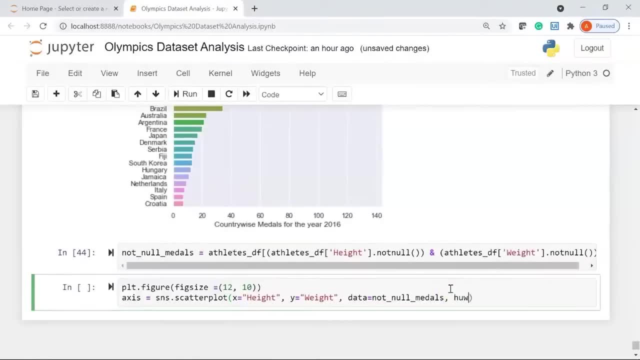 medals comma. i will use hue equal to my sex column- cool. finally, i will say plt dot. i will give a title to my plot saying height versus weight of olympic medalists- olympic medalists- cool. now let's see our scatter plot. this might take some time to. 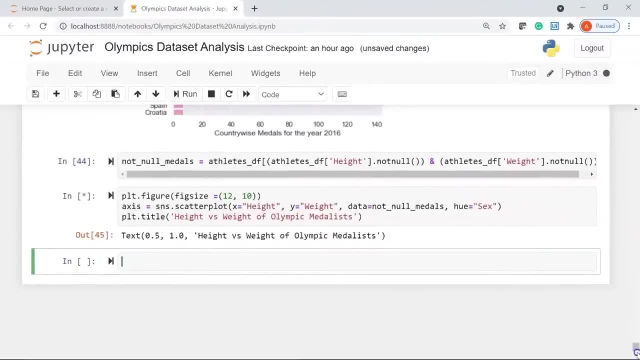 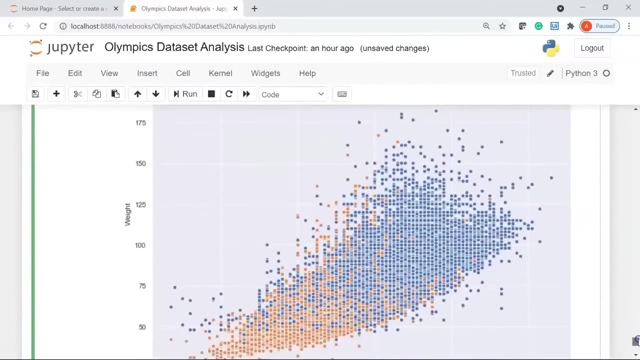 keep the result because there are so many athletes present in a data set who have won a medal, and also we are filtering in terms of hue, which is for male and female. there you go. so if i scroll down, you can see here we have a nice scatter. 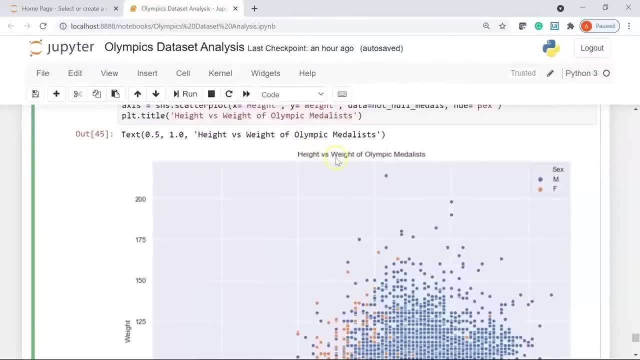 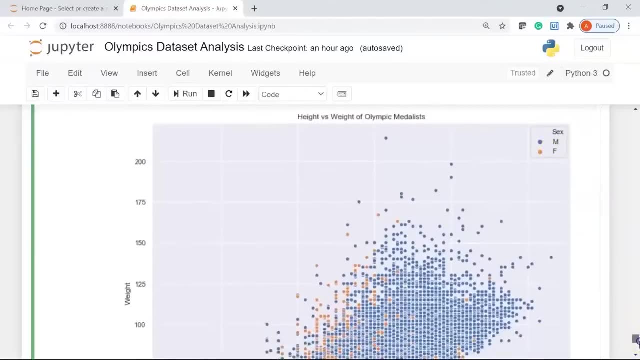 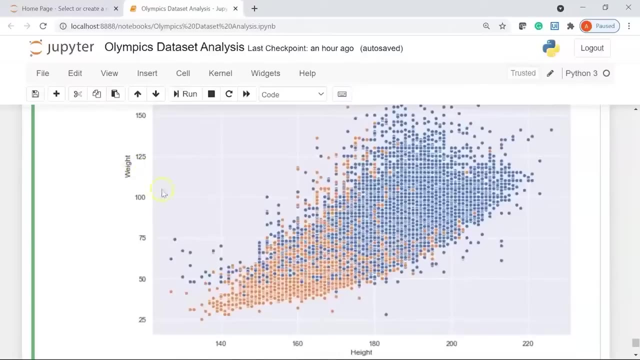 plot. on the top you have the title of the plot saying height versus weight of olympic medalists. you can see our age as the hue. so blue points are for the male athletes and orange points are for the female athletes, and on the y-axis we have the. 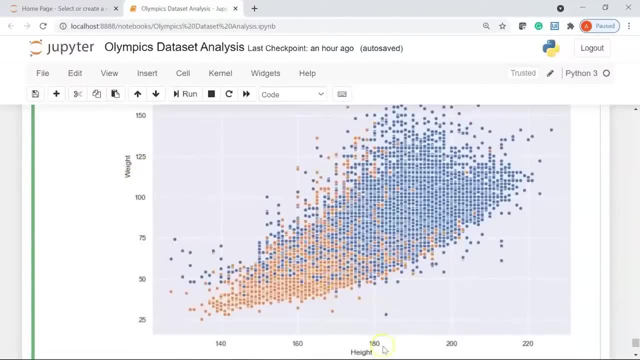 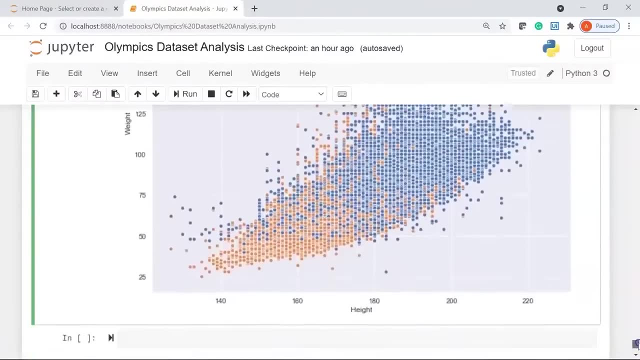 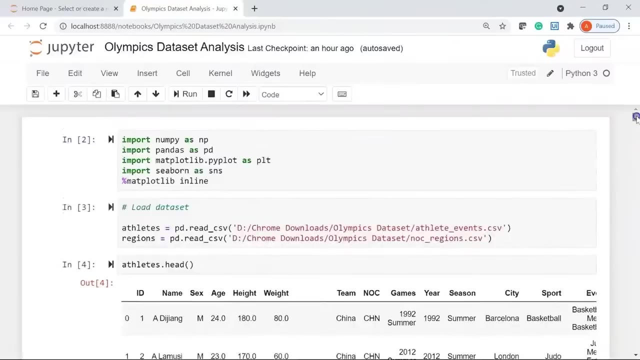 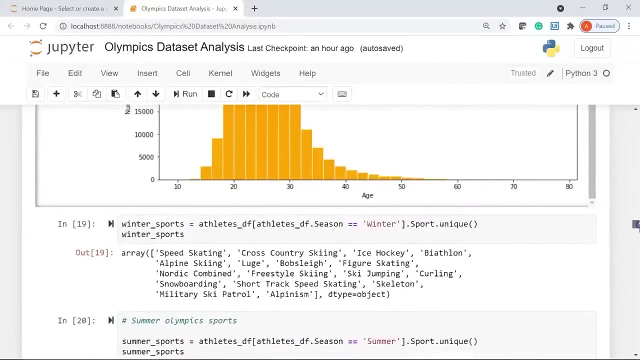 weight in terms of kilograms and you have the height in terms of centimeters. cool. so that brings us to the end of this demo session on olympics data set analysis. so we used two data sets to carry out this exploratory data analysis and we created some. 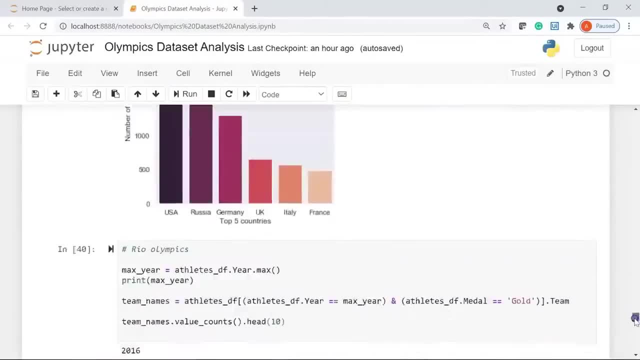 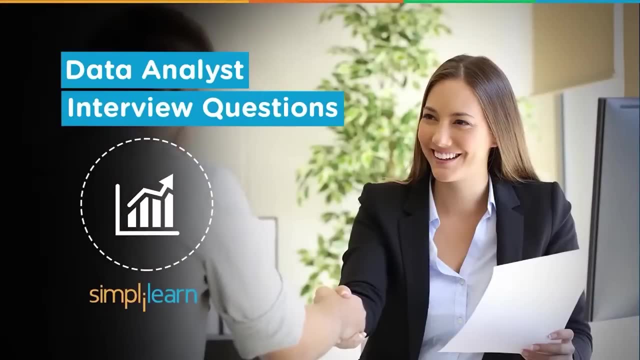 visualizations to analyze and visualize the data. alright, hello and welcome to data analytics interview questions. my name is richard kirschner with the simplylearn team that's wwwsimplylearncom. get certified, get ahead. today we are going to jump into some common questions you might see. 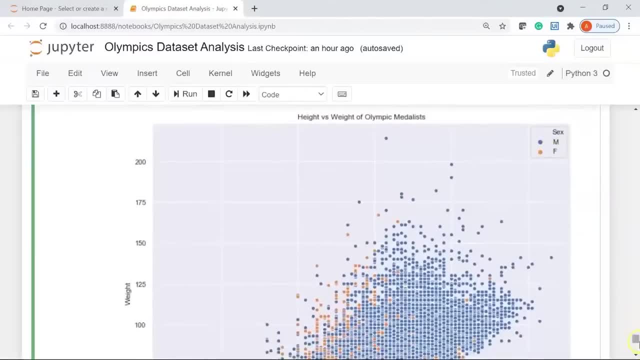 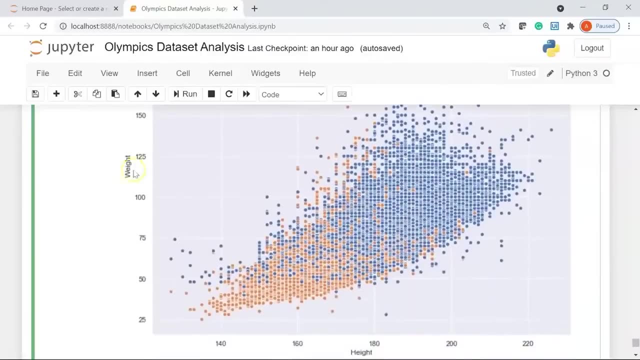 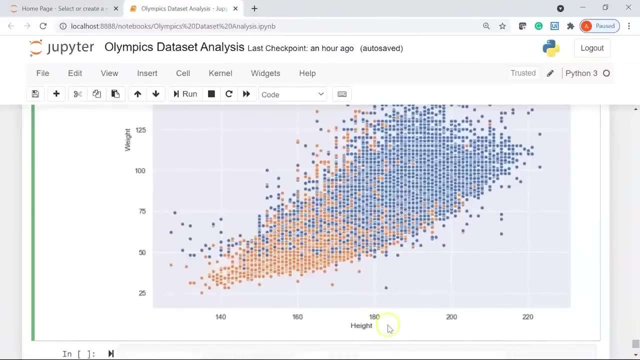 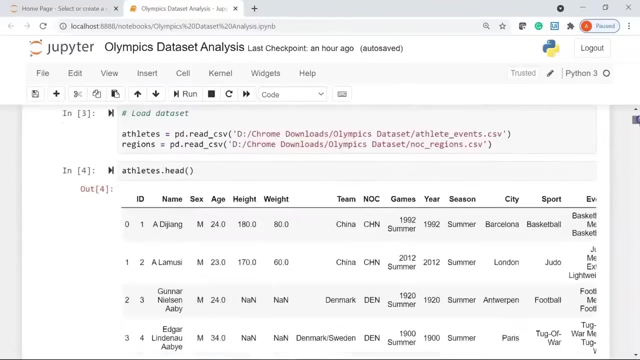 our age as the hue. so blue points are for the male athletes and orange points are for the female athletes, and on the y-axis, we have the weight in terms of kilograms and you have the height in terms of centimeters. cool. so that brings us to the end of this demo session on Olympics data set analysis. so we used 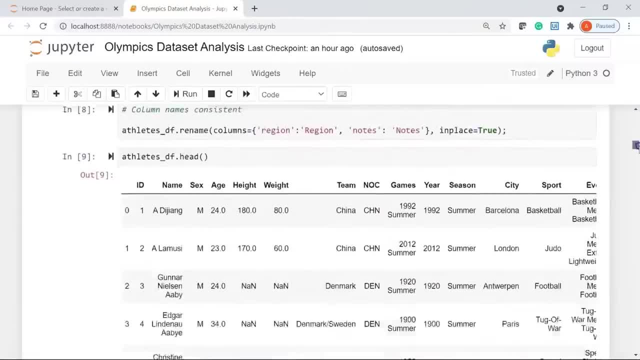 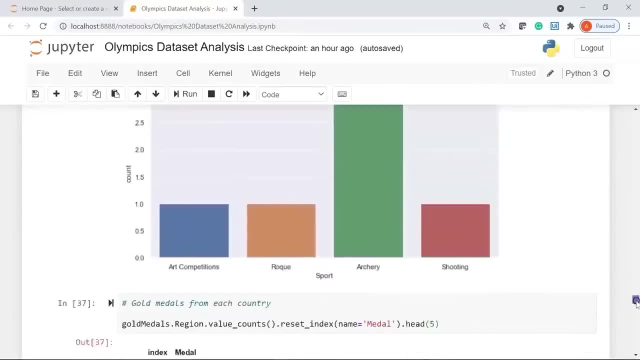 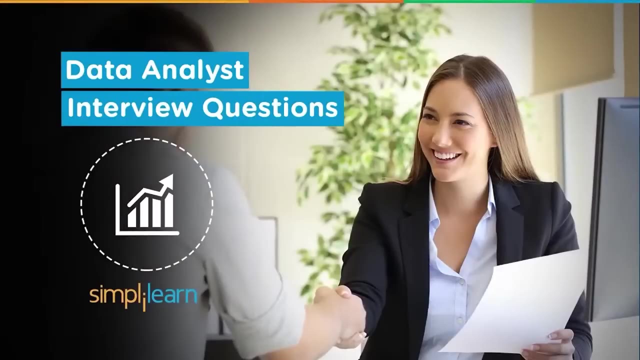 two data sets to carry out this exploratory data analysis and we created some visualizations to analyze and visualize the data. all right, hello and welcome to data analytics interview questions. my name is Richard Kirchner with the simply learn team that's wwwsimplylearncom. get certified, get. 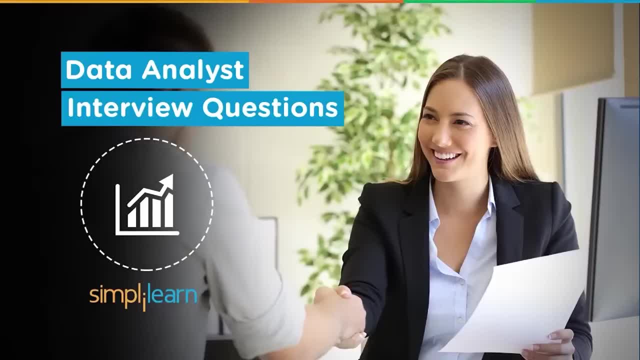 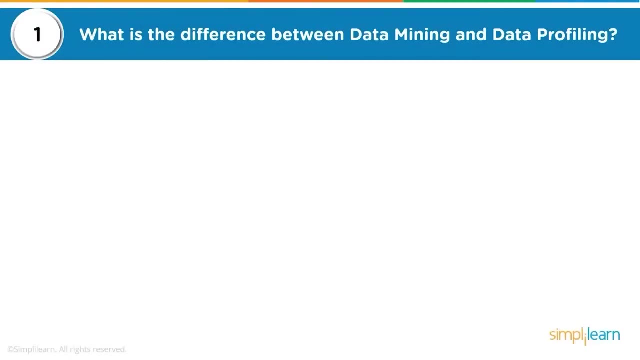 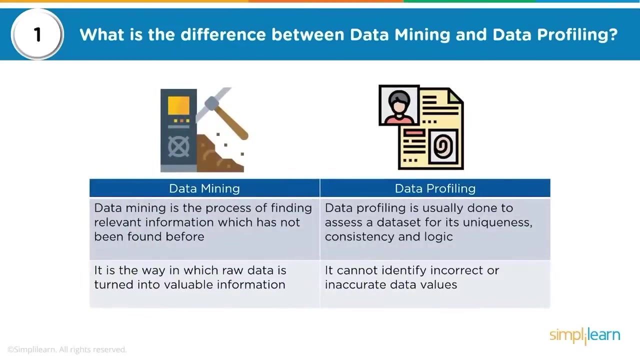 ahead. today we're going to jump into some common questions you might see on numpy, arrays and pandas, data frames in the Python, along with some Excel, tablo and SQL. let's start with our first question: what is the difference between data mining and data analysis, data profiling? it's real important to note that data mining is a process of 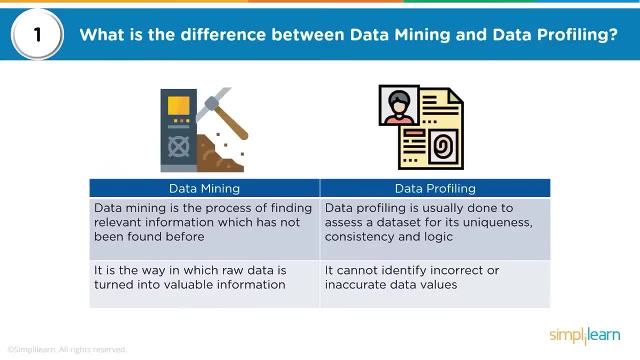 finding relevant information which has not been found before. it is a way in which raw data is turned into valuable information. you can think of this as anything from the cells stats and from their SQL server, all the way to web scraping and Census Bureau information. where the heck do you mine it from where? 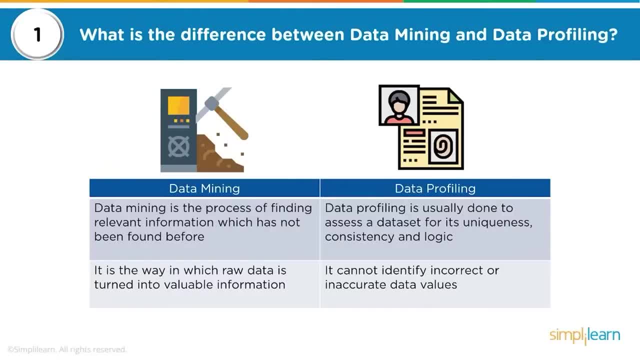 do you get all this data and information? then we look at data profiling. is you're usually done to assess a data set for its uniqueness, consistency and logic. it cannot identify incorrect or inaccurate data values. so if somebody has a statistical analysis on one side and they're doing their, you might in the 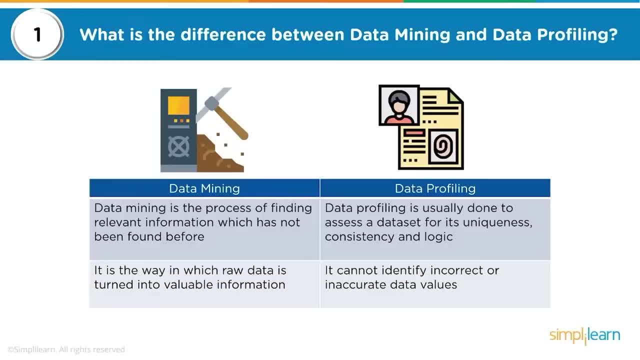 wrong data to then program your data setup. so you got to be aware of that. when you're talking about data mining, you need to look at the integrity of what you're bringing in, where it's coming from. data profiling is looking at it and saying, hey, how is this going to work? what's the logic, what's the? 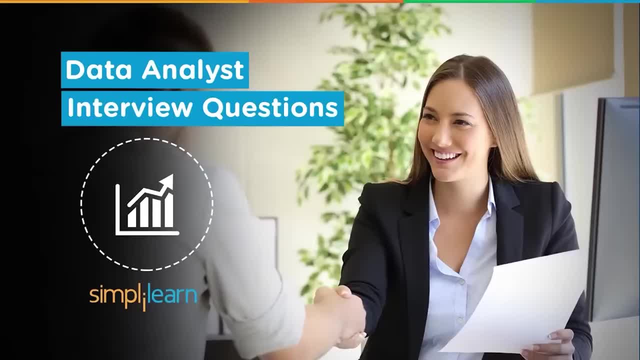 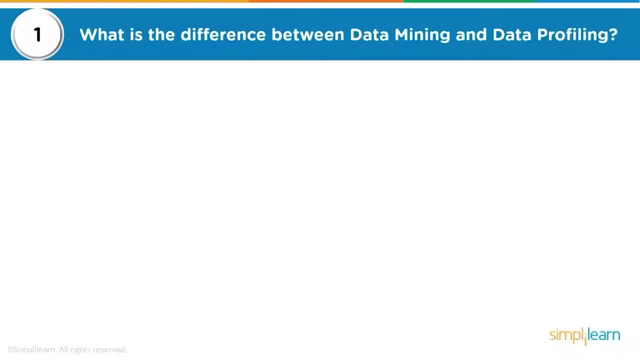 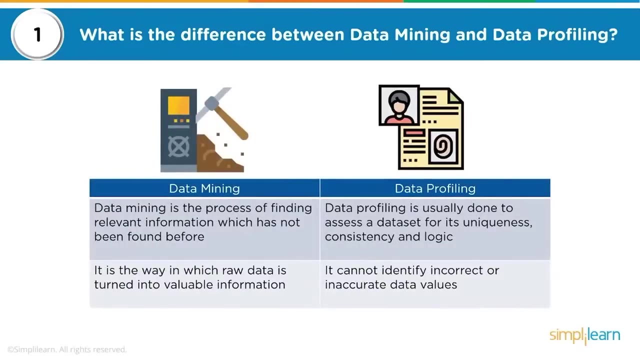 on numpy arrays and pandas, data frames in the python, along with some excel, tablu and sql. let's start with our first question: what is the difference between data mining and data profiling? it's real important to note that data mining is a process of finding relevant information which has not been 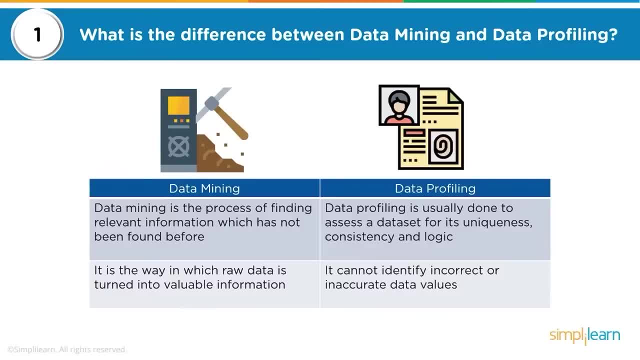 found before. it is a way in which raw data is turned into valuable information. you can think of this as anything from the cells stats and from their sql server all the way to web scraping and census bureau information. where the heck do you mine it? from where do you get all? 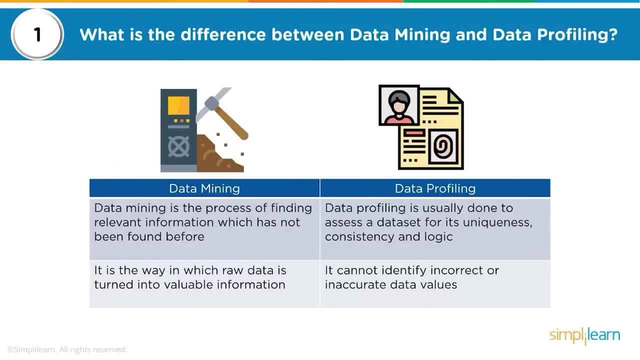 this data and information. then we look at data. profiling is usually done to assess a data set for its uniqueness, consistency and logic. it cannot identify incorrect or inaccurate data values. so if somebody has a statistical analysis on one side and you might be in the wrong data to then program your data, 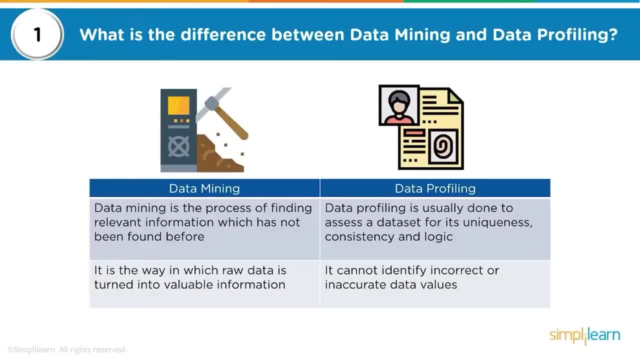 setup. so you got to be aware that when you're talking about data mining, you need to look at the integrity of what you're bringing in, where it's coming from. data profiling is looking at it and saying, hey, how is this going to work? what's the logic, what's the consistency? 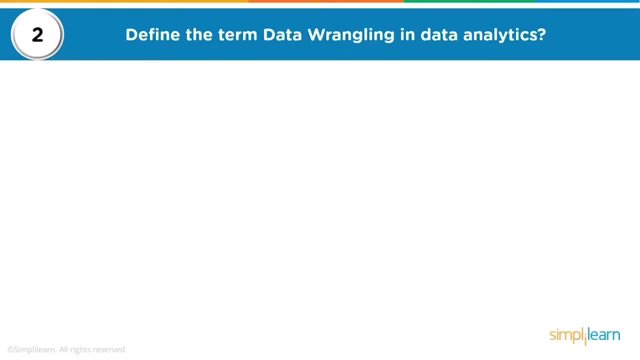 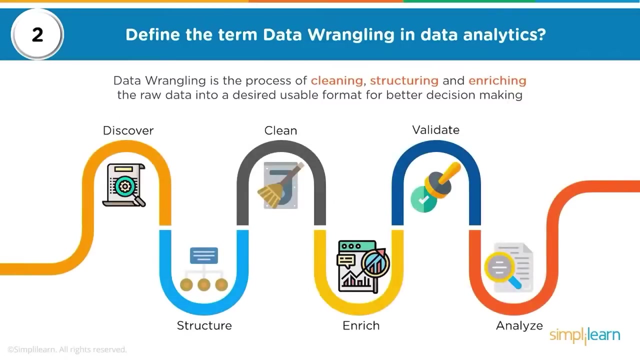 is it related to what i'm working with? find the term data wrangling and data analytics. data wrangling is a process of cleaning, structuring and enriching the raw data into a desired usable format for better decision making, and you can see a nice chart here with our discover it. 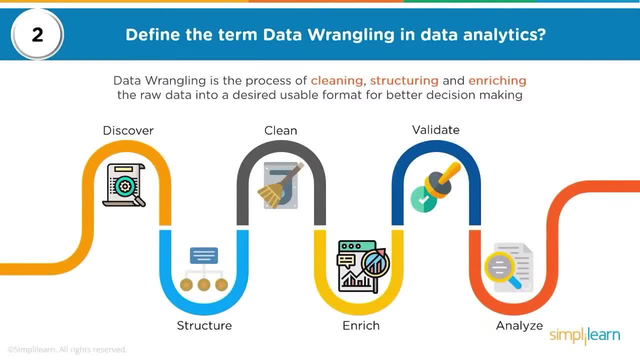 we structure the data how we want it. we clean it up, get rid of all those null values, we enrich it so we might take and reformat some of the settings, instead of having five different terms for height of somebody you know, in american, english or whatever. we clean some of that up and we might do a calculation. 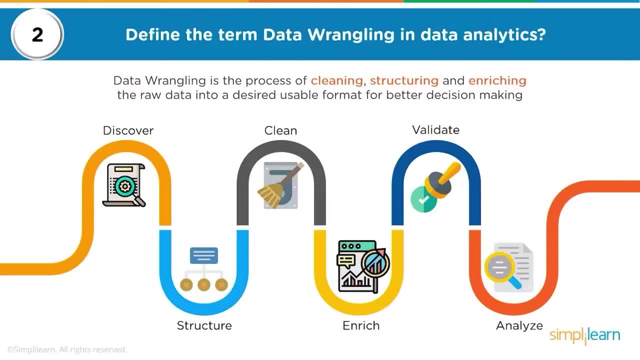 and bring some of them together and validate. i was just talking about that in the last one. you need to validate your data, make sure you have a solid data source and then, of course, it goes into the analysis. very important to notice here in data wrangling: eighty percent of data analytics. 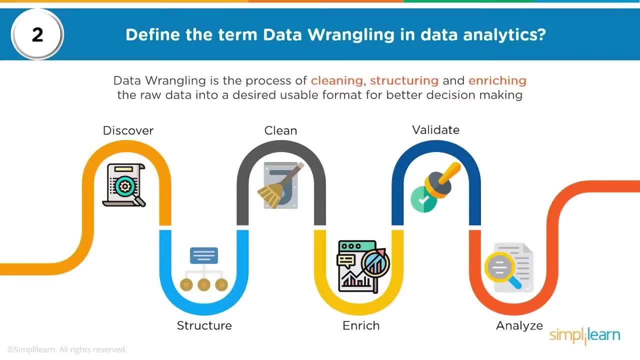 is usually in this whole part of wrangling the data, getting it to fit correctly, and don't confuse that with data cooking, which is actually when you're going into neural networks cooking the data. so it's all between zero and one values. what are common problems that data analysts? 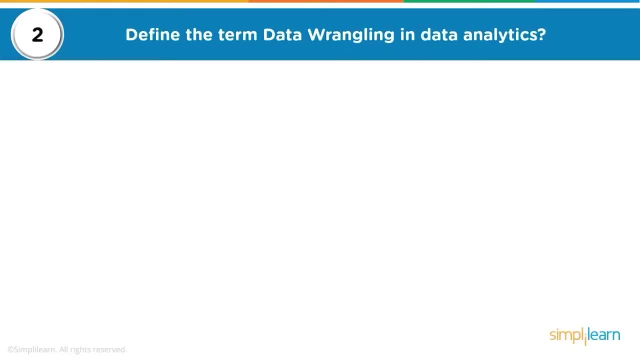 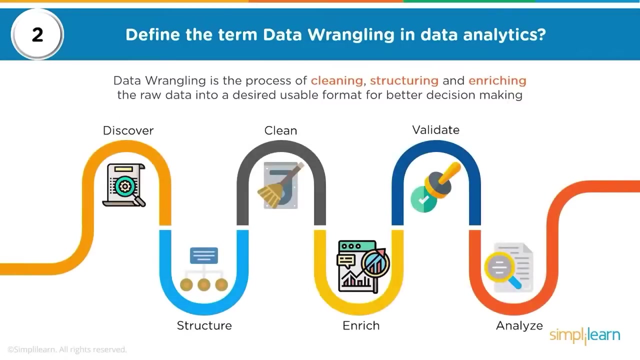 consistency. is it related to what I'm working with? find the term data wrangling and data analytics. data wrangling is a process of cleaning, structuring and enriching the raw data into a desired usable format for better decision-making, and you can see a nice chart here with our discover. 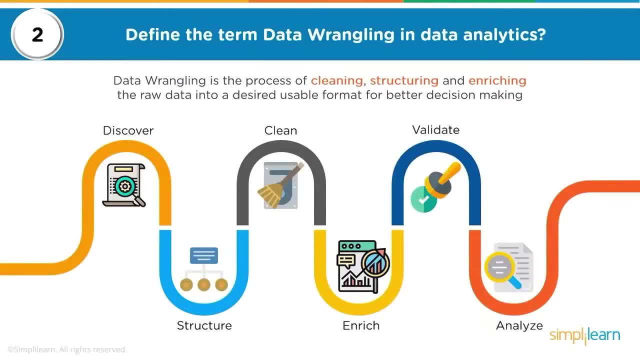 it. we just structure the data how we want it. we clean it up, get rid of all those null values. we enrich it so we might take in, reformat some of the settings, instead of having five different terms for height of somebody, you know, in American, English or whatever. 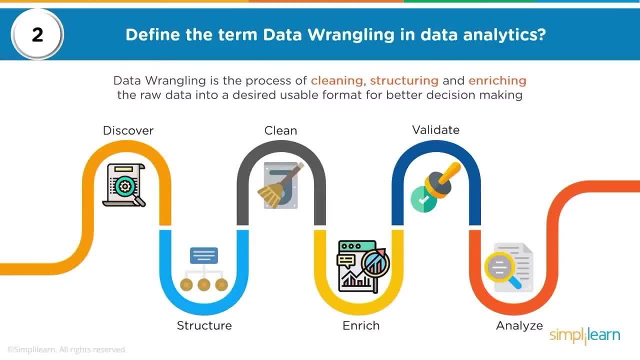 some of that up and we might do a calculation and bring some of them together and validate. i was just talking about that in the last one. you need to validate your data, make sure you have a solid data source and then of course, it goes into the analysis- very important to notice here in data. 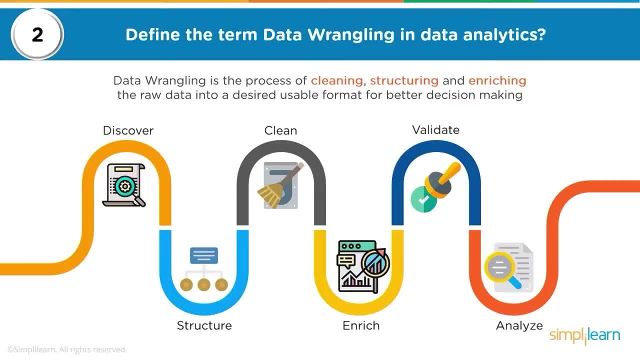 wrangling 80 of data analytics is usually in this whole part of wrangling the data, getting it to fit correctly. and don't confuse that with data cooking, which is actually when you're going into neural networks cooking the data. so it's all between zero and one values. what are common problems that? 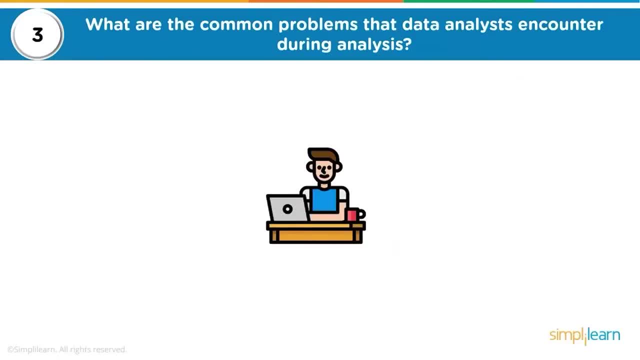 data analysts encounter during analysis: handling duplicate and missing values, collecting the meaningful, right data the right time. making data secure and dealing with compliance issues, handling data purging and storage problems. again we're talking about data wrangling here. 80 of most jobs are in wrangling that data and getting 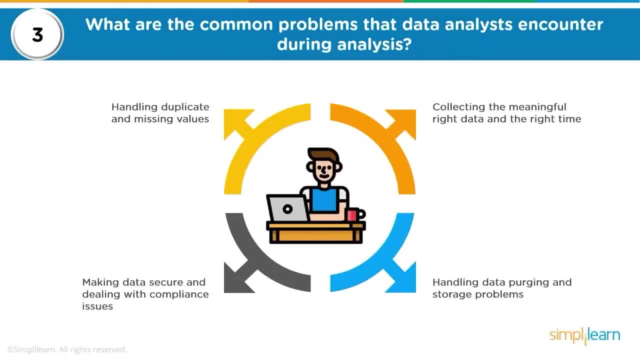 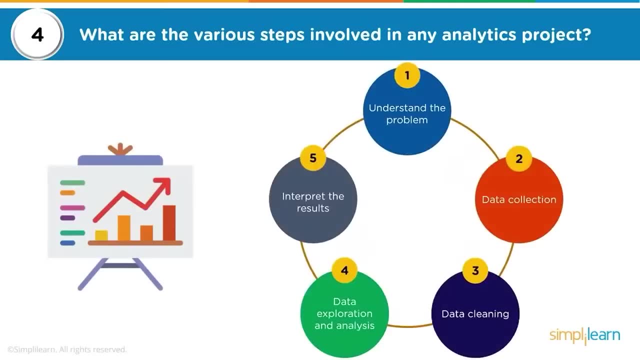 it in the right format and making sure it's good data to use. number four: what are the various steps involved in any analytics project? understand the problem. we might spend 80 percent doing wrangling, but you better be ready to understand the problem because if you can't, you're going to spend all your time in the wrong direction. this is probably the most. 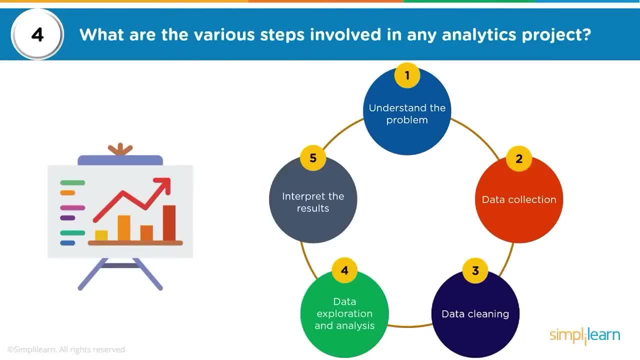 important part of the process, everything after it falls in and then you can come back to it. two: data collection, data cleaning. number three, four: data exploration, analysis. and five: interpret the results. number five is a close second for being the most important. if you can't interpret what you bring to the table to your clients, you're in trouble. 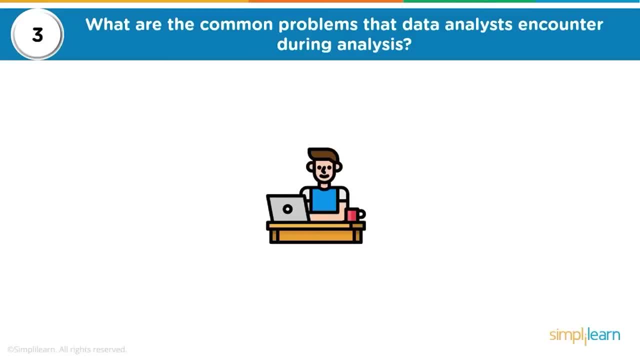 encounter during analysis: handling duplicate and missing values, collecting the meaningful, right data the right time, making data secure and dealing with compliance issues, handling data purging and storage problems. again, we're talking about data wrangling here. eighty percent of most jobs are in wrangling that data and 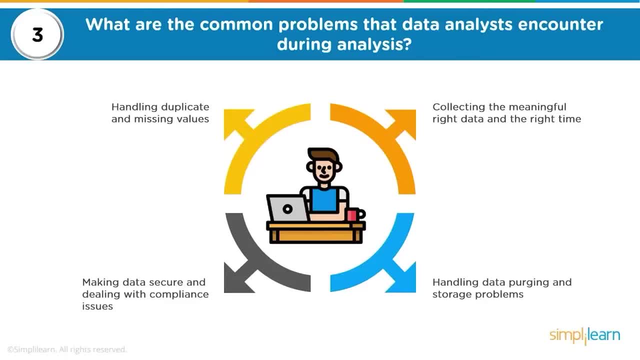 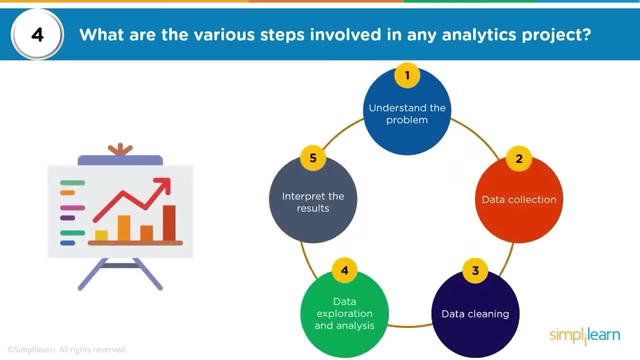 getting it in the right format and making sure it's good data to use. number four: what are the various steps involved in any analytics project? understand the problem. we might spend eighty percent doing wrangling, but you better be ready to understand the problem because if you can't, you're. 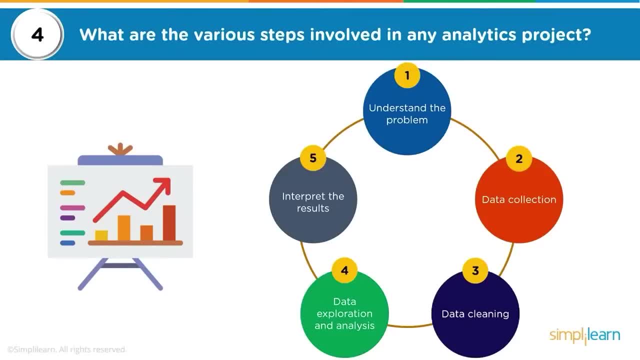 going to spend all your time in the wrong direction. this is probably the most important part of the process: everything after it falls in and then you can come back to it. two: data collection, data cleaning. number three. four: data exploration analysis. and five: interpret the results. number five is a close second for being the most. 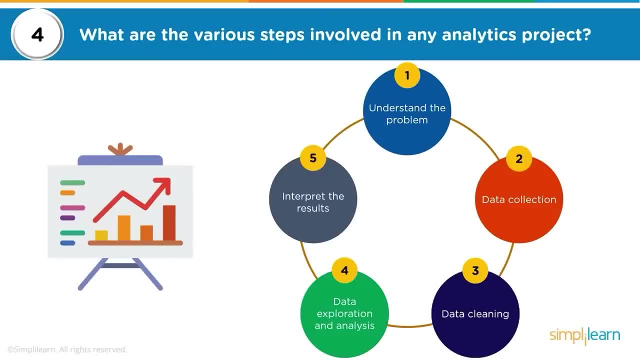 important. if you can't interpret what you bring to the table to your clients, you're in trouble. so when you this question comes up, you probably want to focus on those two, noting that the rest of it does. eighty percent of the work is in two, three and four. well, one, 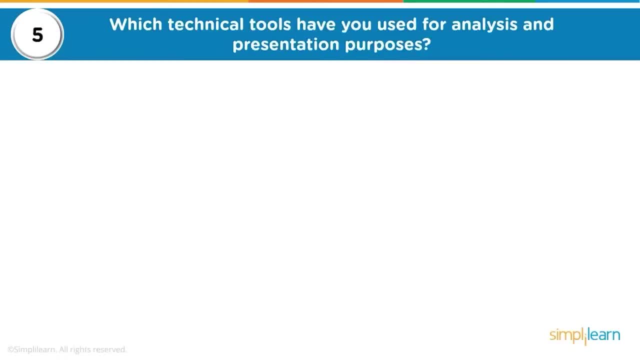 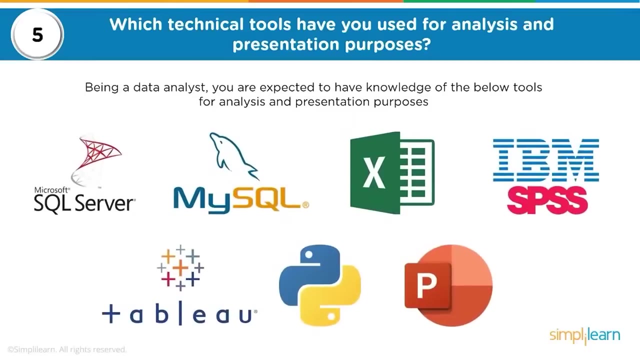 and five are the most important parts. which technical tools have you used for analysis and presentation purposes? being a data analyst, you are expected to have knowledge of the below tools for analysis and presentation purposes. there's a wide variety out there: sql server, mysql. you have your excel, your. 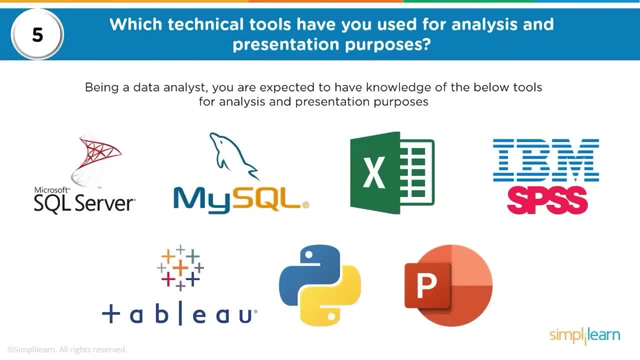 spss, which is the ibm platform, tableau, python- you have all these different tools in here now. certainly a lot of jobs are going to be narrowed in on just a few of these tools. like you're not going to have a microsoft sql server, mysql server, but you better understand. 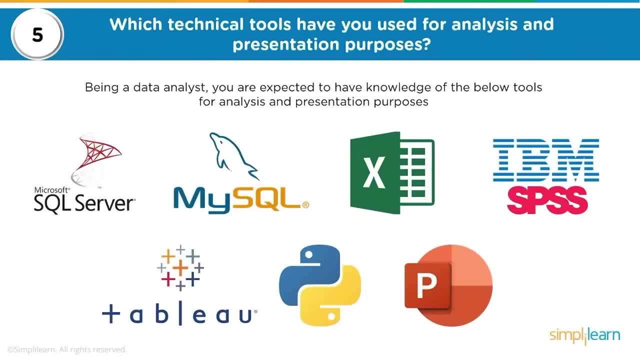 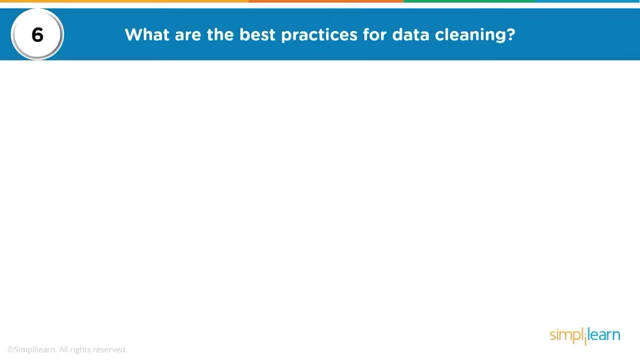 how to do basic sql polls and also understanding excel and how, the different formats for column and how to get those set up. number six: what are the best practices for data cleaning? this is really important to remember to go through this in detail. these always come up because eighty percent. 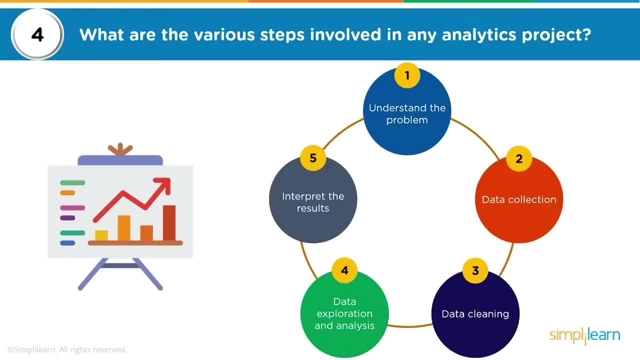 so when this question comes up, you probably want to focus on those two, noting that the rest of it does. 80 of the work is in two, three and four. well, one and five are the most important parts. so the first thing to do is to analyze what's in the list. there are a couple of tools on here. 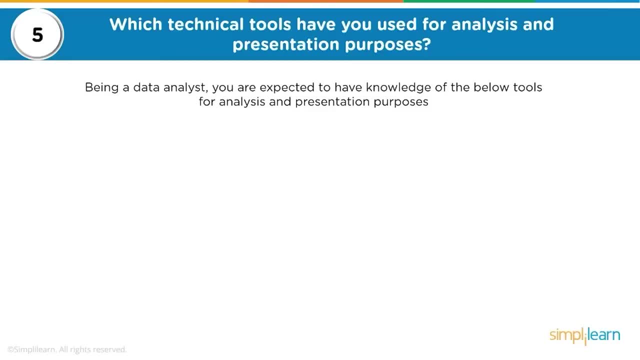 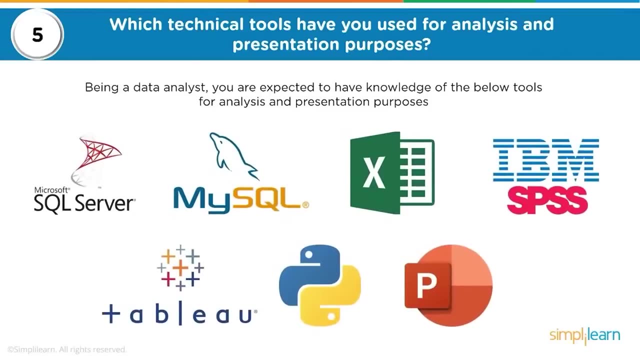 the first one is to use the search engine. so search engine is one of the most useful tools that you have across your entire system. so if you're going to use it on your phone and you need it to be in active use, you can use it for whatever you want. so, for example, you can use it to search: 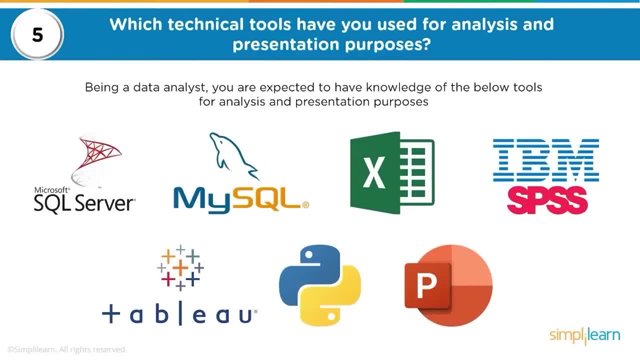 your device. you can use it to search your mobile or to run a workstation. now the second key is to use the search engine. so if you're using aовалi search engine, there is a lot of tools you must use. so a Microsoft SQL Server, my SQL Server, but you better understand how to do basic SQL polls. 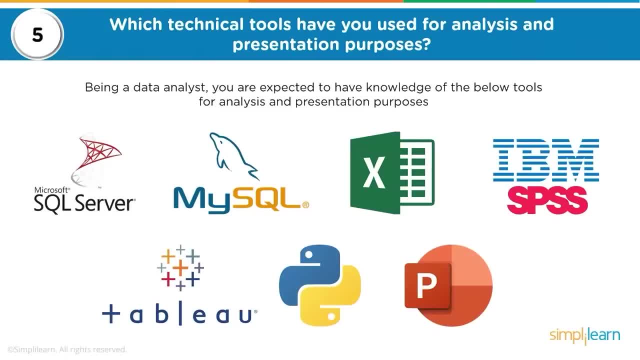 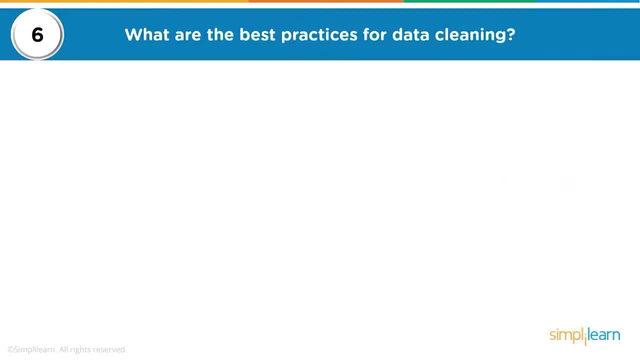 and also understanding Excel and how, the different formats from column and how to get those set up. number six: what are the best practices for data cleaning? this is really important to remember to go through this in detail. these always come up because 80% of most data analysis is in cleaning. 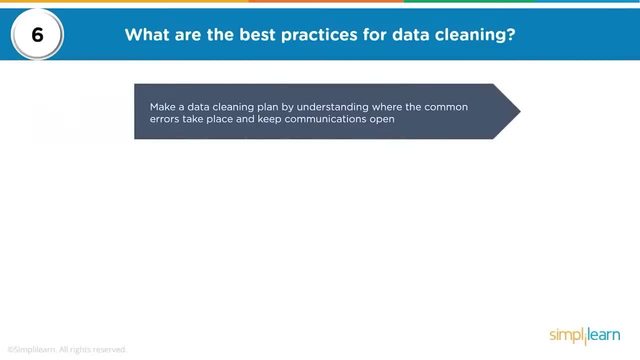 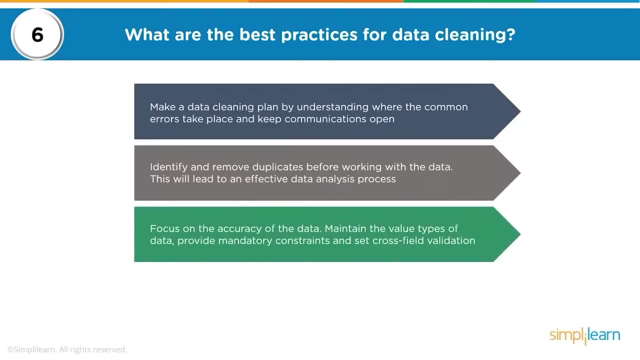 the data. make a data cleaning plan by understanding where the common errors take place and keep communications open. identify and remove duplicates before working with the data. this will lead to an effective data analysis process. focus on the accuracy of the data. maintain the value types of data. provide mandatory constraints and set cross field validation. standardize the data at. 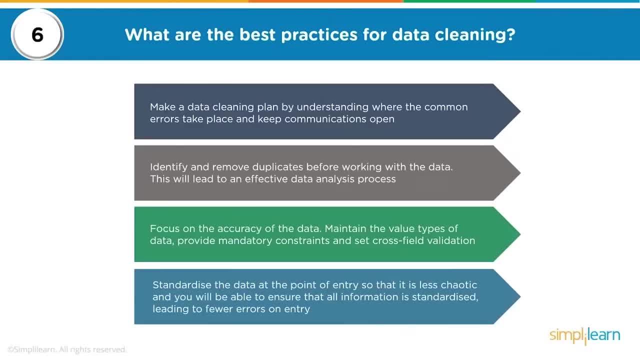 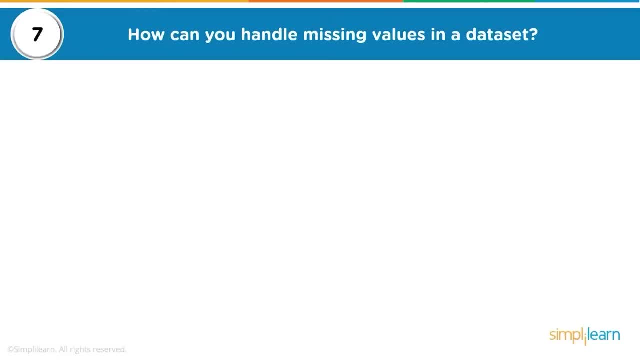 the point of entry, so that is less chaotic and you will be able to ensure that all the information is standardized, leading to future data cleaning processes. next slide, please, number seven: how can you handle missing values in a data set, listwise deletion and listwise deletion method: entire record is excluded from analysis if any single value is missing. sometimes we're 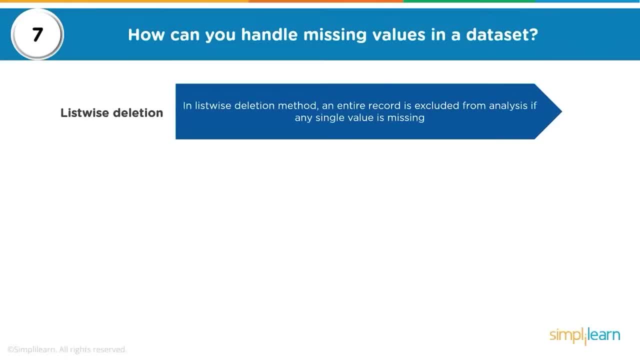 talking about records, remember this could be a single line in a database. so if you have, your SQL comes back and you have 15 different columns, every one of those has a missing value. you might just drop it just to make it easy, because you already have enough data to do the process. 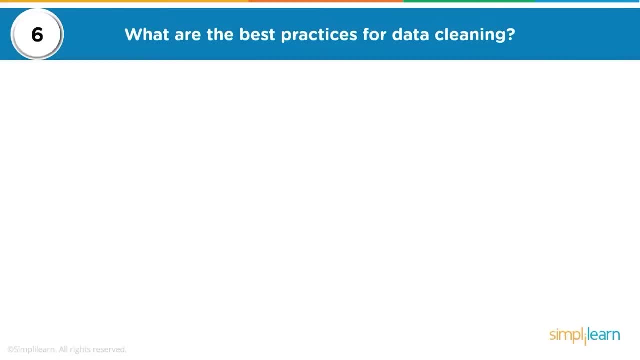 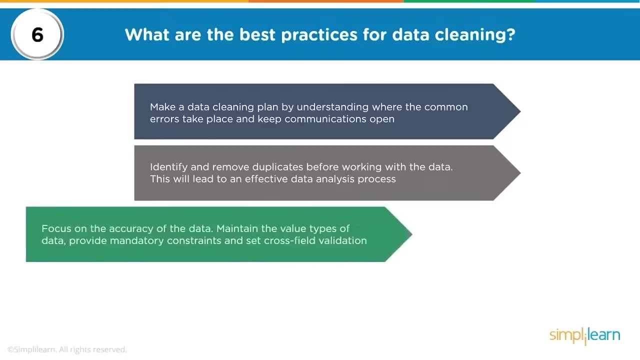 of most data analysis is in cleaning the data. make a data cleaning plan by understanding where the common errors take place and keep communications open. identify and remove duplicates before working with the data. this will lead to an effective data analysis process. focus on the accuracy of the data. maintain the 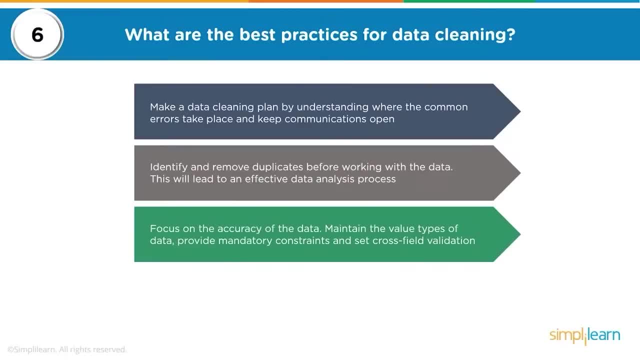 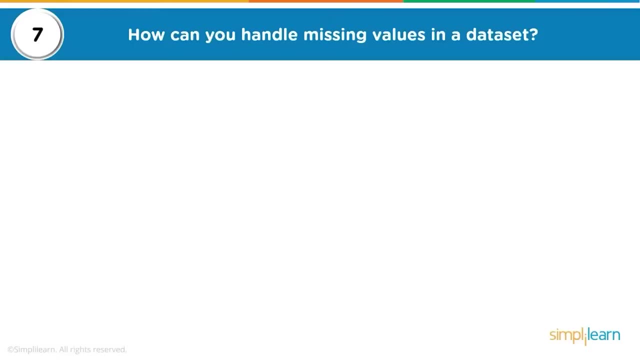 value types of data, provide mandatory constraints and set cross field validation. standardize the data at the point of entry so that it is less chaotic and you will be able to ensure that all the information is standardized, leading to fewer errors. on entry number seven, how can you handle? 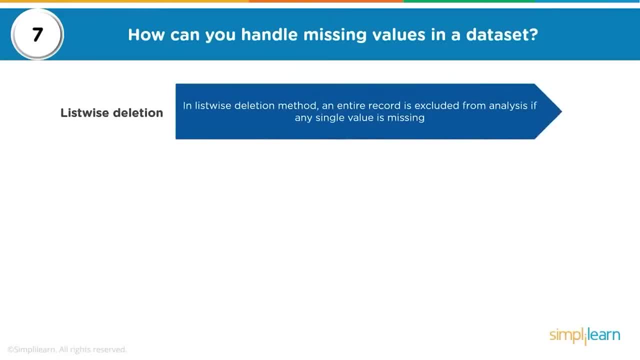 missing values in a data set list: wise deletion. in list wise deletion method, entire record is excluded from analysis if any single value is missing- sometimes we're talking about records, remember this could be a single line in a database. so if you have, your sql comes back and you have. 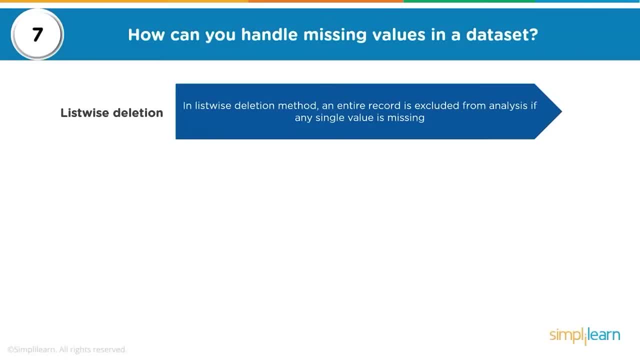 fifteen different columns. every one of those has a missing value. you might just drop it just to make it easy, because you already have enough data to do the processing average imputation. use the average value of the responses from the other participants to fill in the missing value. 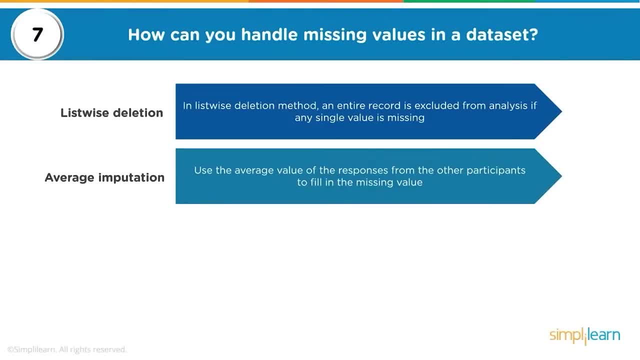 this is really useful, and they'll ask you why these are useful. i guarantee it. if you have a whole group of data that's collected and it doesn't have that information in it, at that point you might average it in there. regression substitution: you can use multiple regression analysis to estimate. 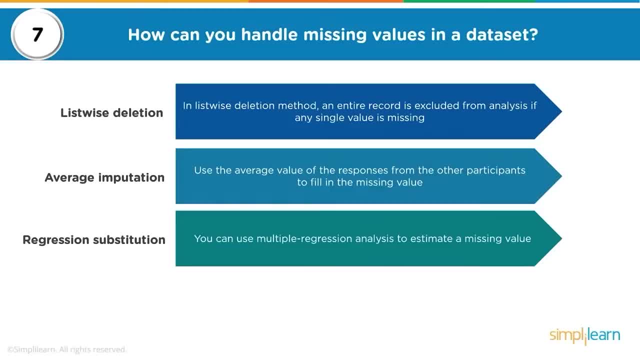 a missing value. that kind of goes with the average imputation. input regression model means you're just going to get, you're going to actually generate a prediction as to what you think that value should be for those people, based on the ones you do have multiple imputation. so we're talking. 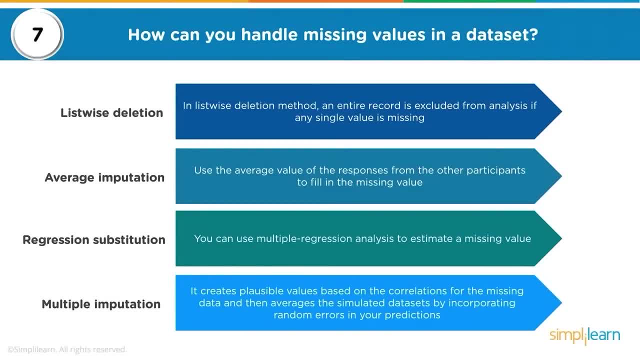 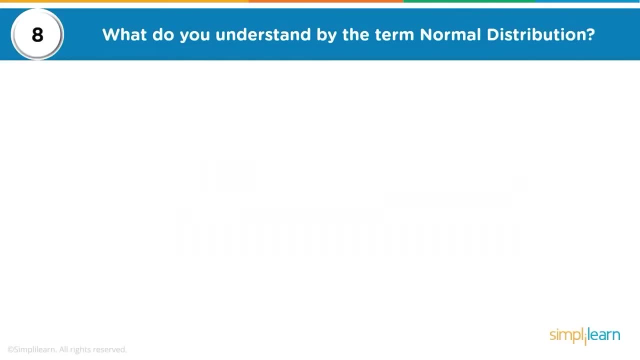 about multiple inputs. it creates plausible values based on the correlations for the missing data and then average the simulated data sets by incorporating random errors in your calculations. what do you understand by the term normal distribution? and the second you hear the word normal distribution should be thinking a bell. 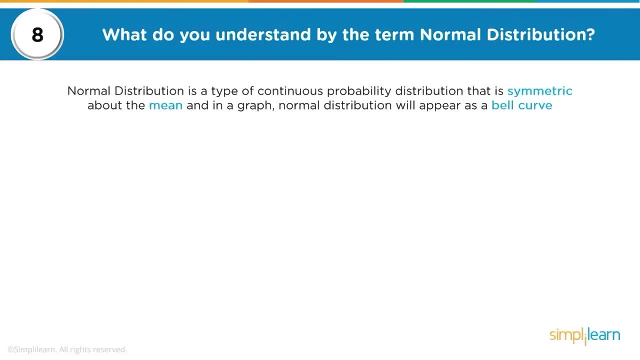 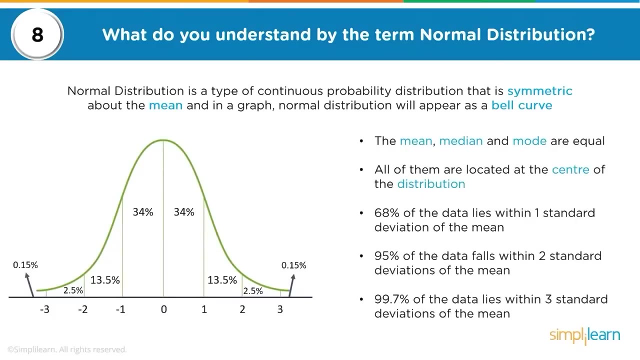 curve like we see here. normal distribution is a type of continuous probability distribution that is symmetric about the mean and in the graph normal distribution will appear as a bell curve. the mean, median and mode are equal. that's a quick way to know if you have normal distribution is you can compute. 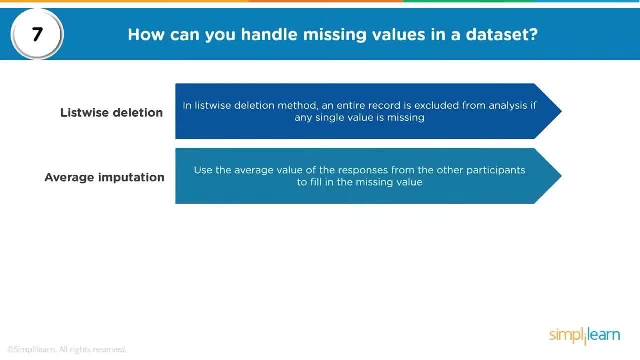 average imputation. use the average value of the responses from the other participants to fill in the missing value. this is really useful and they'll ask you why these are useful. I guarantee it. if you have a whole group of data that's collected and it doesn't have that information, 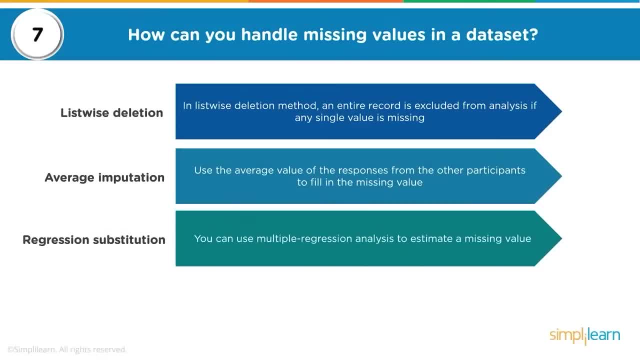 in it. at that point you might average it in their regression substitution. you can use multiple regression analysis to estimate a missing value. that kind of goes with the average imputation input. regression substitution is very common in data sets such as the first one. if you are not an 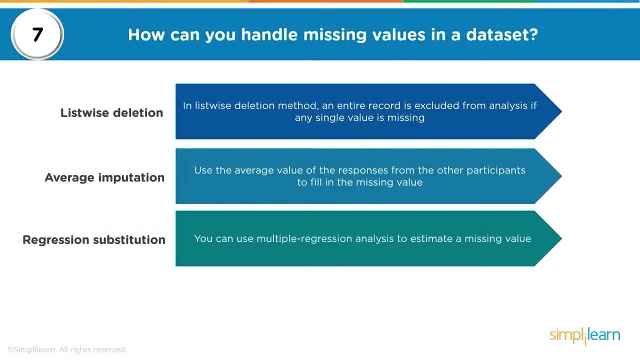 input, you're typically going to have a missing value. if you are an input, you're probably going to have a missing value. you're probably going to have a missing value. if you're not an input, you're model means you're just going to get. you're going to actually generate a prediction as to what you. 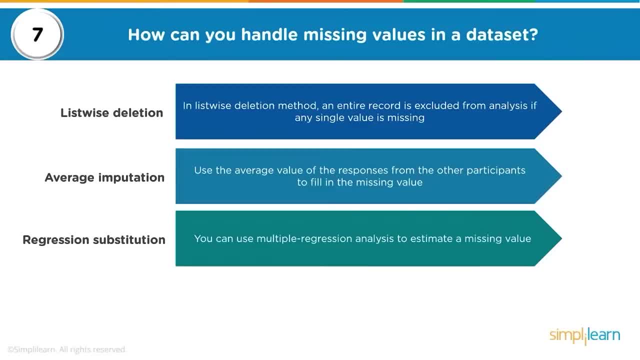 think that value should be for those people based on the ones. you do have multiple imputation, so we talk about multiple inputs. it creates plausible values based on the correlations for the missing data and then average the simulated data sets by incorporating random errors in your predictions. what do you understand by the term normal distribution? and the second you hear the. 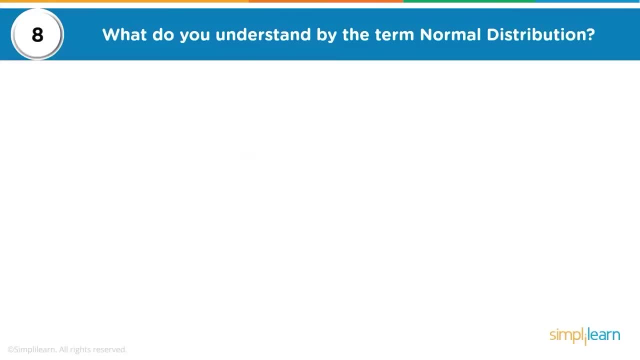 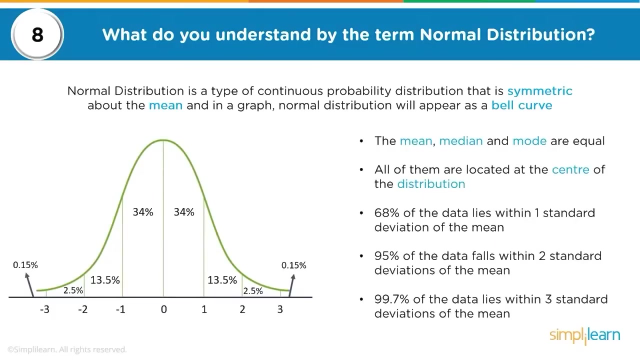 word normal distribution should be thinking of bell curve. like we see here, normal distribution is a type of continuous probability distribution that is symmetric about the mean, and in the graph normal distribution will appear as a bell curve. the mean, median and mode are equal. that's a quick way to know if you have normal distribution is you can compute mean, median and. 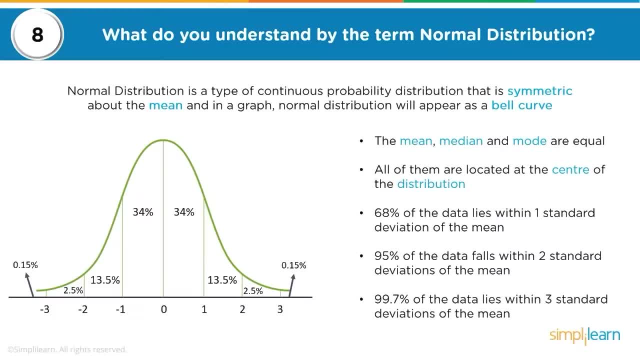 mode. all of them are located at the center of the distribution. 68 of the data lies within one standard deviation of the mean 98. a sky middle position of a value 應該 term pensions of villainy numberstation of 0.15 million. individual CaptURE Pe 모르p strongly. 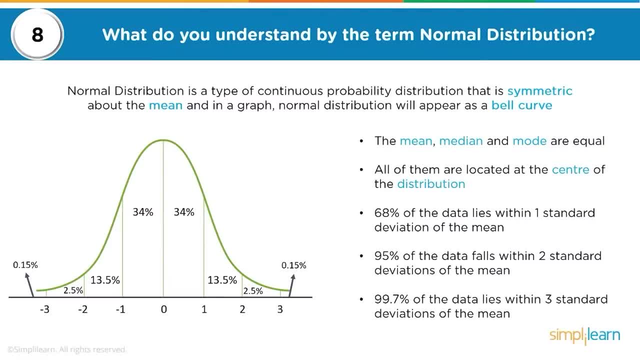 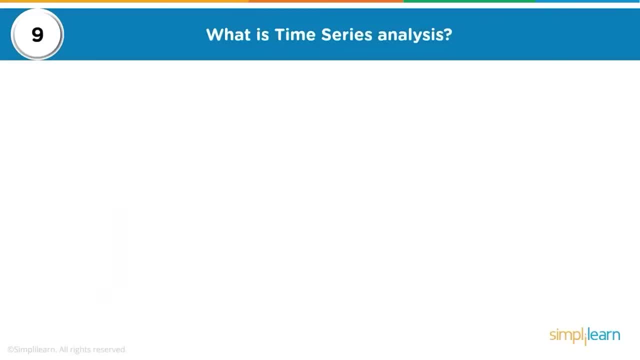 95% of the data falls within two standard deviations of the mean. 99.7% of the data lies within three standard deviations of the mean. What is time series analysis? Time series analysis is a statistical method that deals with ordered sequence of values. 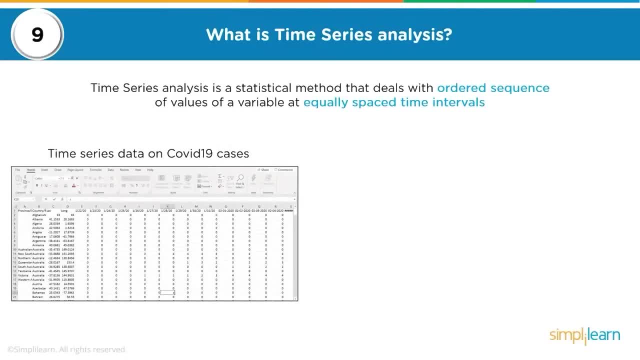 of a variable of equally spaced time intervals, Time series data on a COVID-19 cases, and you can see we're looking at by days. so our space is of days and each day goes by. If we take and graph it, you can see a time series graph always looks really nice if 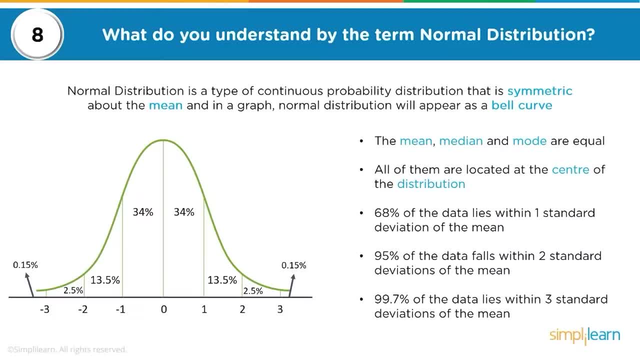 mean, median and mode. all of them are gonna be in the center of the distribution. sixty-eight percent of the data lies within one standard deviation of the mean. ninety-five percent of the data falls within two standard deviations of the mean. ninety nine point seven percent of the data lies. 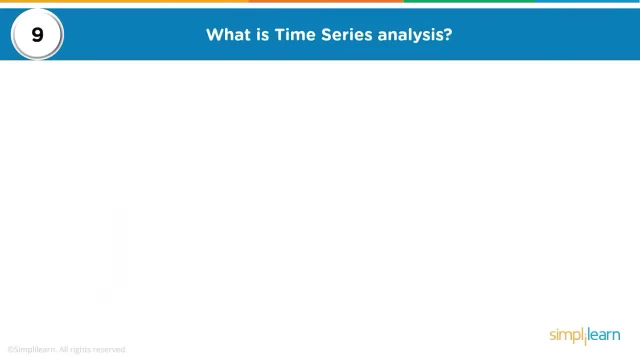 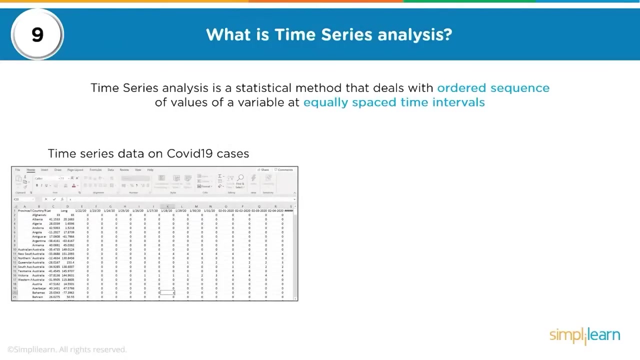 within three standard deviations of the mean. what is time series analysis? time series analysis is a statistical method that deals with ordered sequence of values of a variable of equally spaced time intervals- time series data on a certain time series data is a covid- 19 cases and you can see we're looking at by days. so our space is of days and each day goes by. 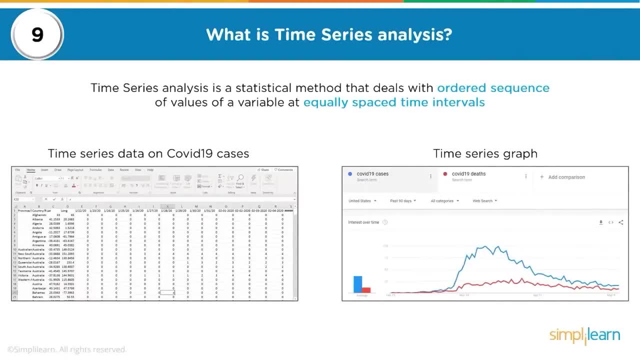 if we take and graph it, you can see a time series. graph always looks really nice if you have like two different. in this case, we have what- the united states going over there. i'd have to look at the other setup in there, but they picked a couple different countries. uh, and it is it's time. 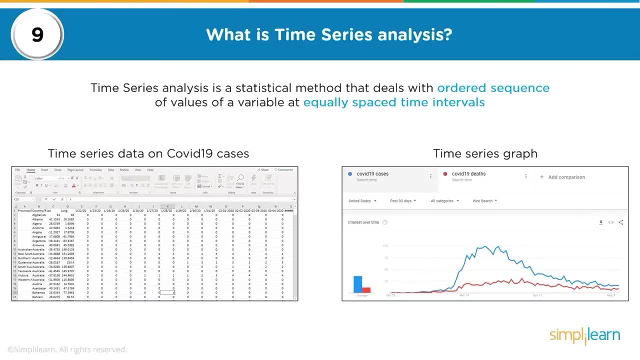 sensitive: yeah, with. the next result is based on what the last one was. kobe is an excellent example of this. anytime you do any word analytics- where you're figuring out what someone's saying, what they said before, makes a huge difference- is what they're going to say next- another form of time. 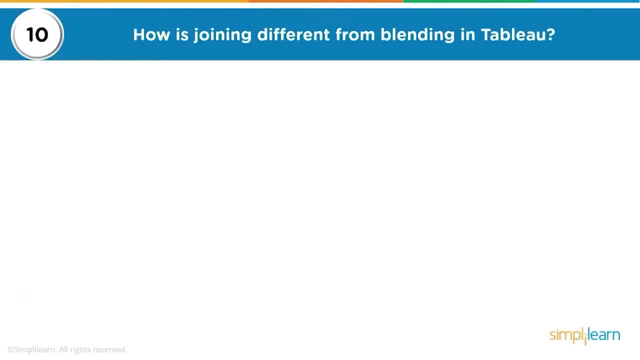 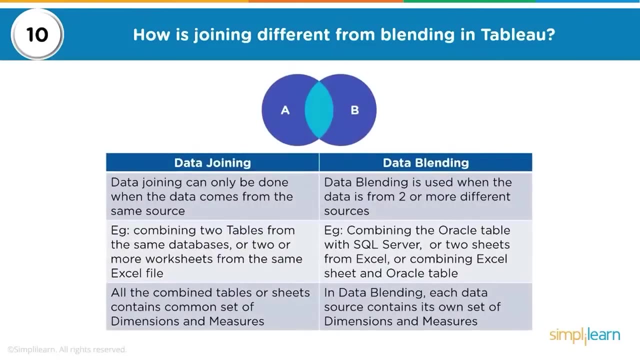 series analysis 10.. how is joining different from blending in tableau? so now we're going to jump into the tableau package: data joining: data joining can only be done when the data comes from the same source: combining two tables from the same database or two or more worksheets from 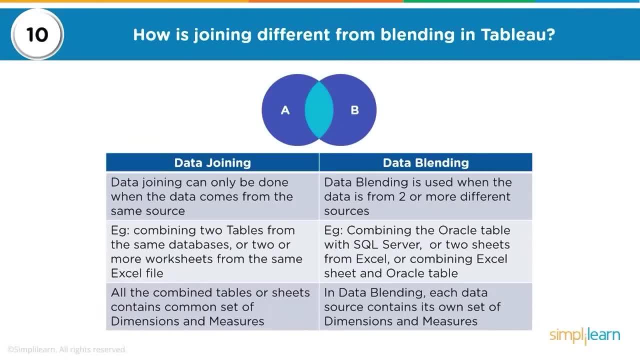 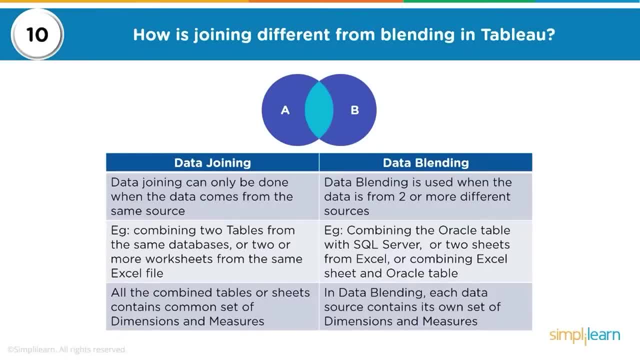 sheets contains common set of dimensions. sheets contains common set of dimensions and measures. data blending: data blending and measures. data blending: data blending and measures. data blending: data blending is used when the data is from two or more. is used when the data is from two or more. is used when the data is from two or more different sources. combining the oracle. 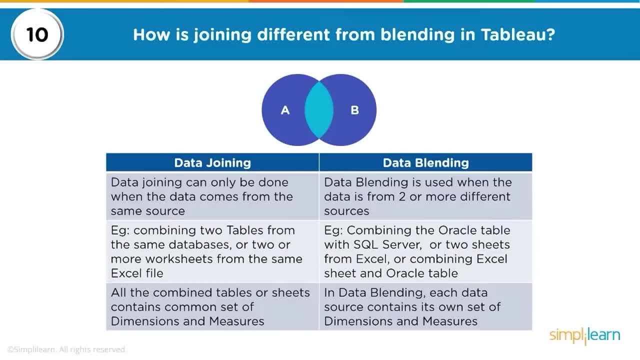 different sources. combining the oracle. different sources. combining the oracle table with the sql server. or two sheets table with the sql server or two sheets table with the sql server, or two sheets from excel or combining excel sheet and from excel, or combining excel sheet and from excel, or combining excel sheet and oracle table in data blending each data. 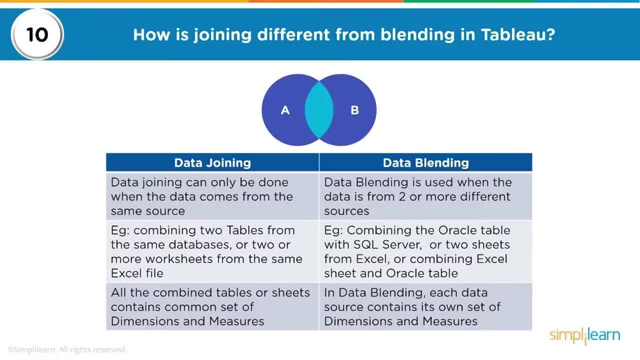 oracle table in data blending. each data oracle table in data blending. each data source contains its own set of source, contains its own set of source. contains its own set of dimensions and measures. dimensions and measures. dimensions and measures. how is overfitting different from? how is overfitting different from? 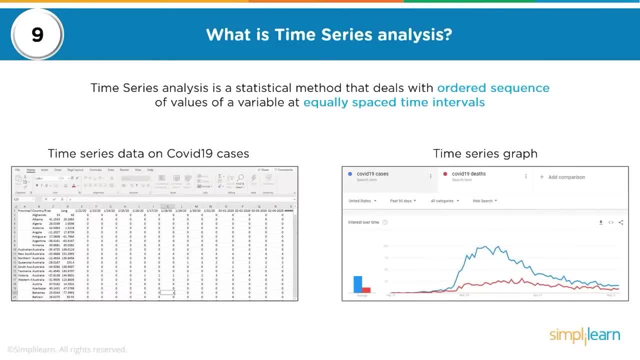 you have like two different. in this case we have what the United States going over there. I'd have to look at the other setup in there, but they picked a couple of different countries And it is it's time sensitive, you know, with. the next result is based on what the 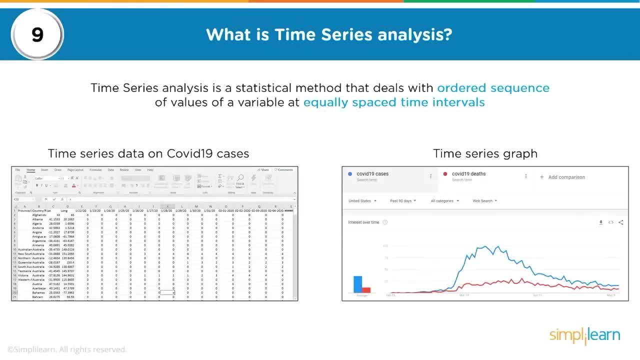 last one was COVID is an excellent example of this. Anytime you do any word analytics, where you're figuring out what someone's saying, what they said before makes a huge difference. That's what they're going to say next, another form of time series analysis. 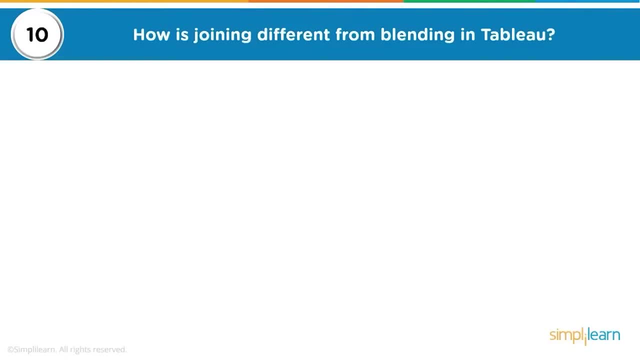 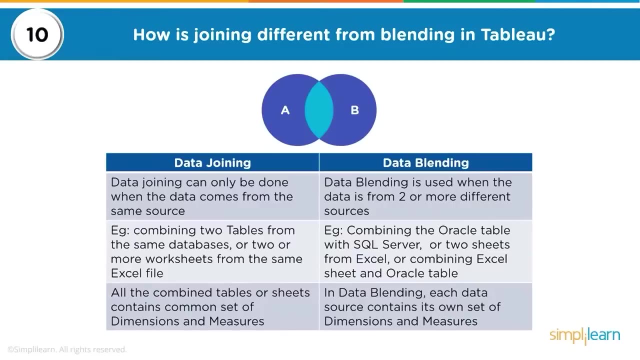 10. How is joining different from blending in Tableau? So now we're going to jump into the Tableau package: Data joining: Data joining can only be done when the data comes from the same source, Combining two tables from the same database or two or more worksheets from the same Excel. 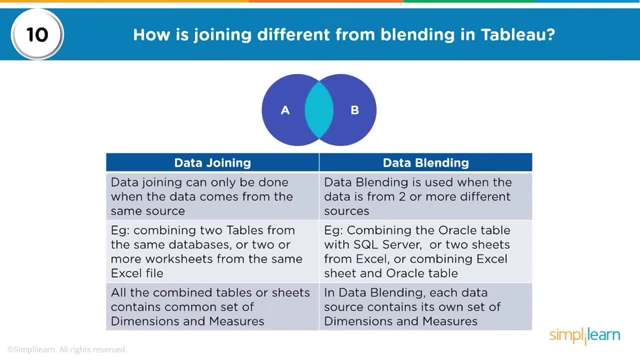 file- All the combined tables or sheets- contains common set of dimensions and measures. 10. Data blending. Data blending is used when the data is from two or more different sources: Combining the Oracle table with the SQL server or two sheets from Excel or combining Excel. 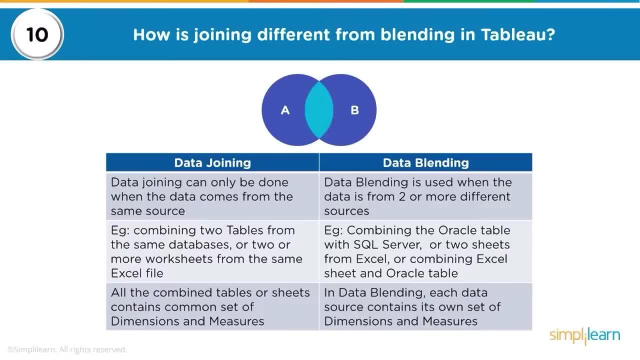 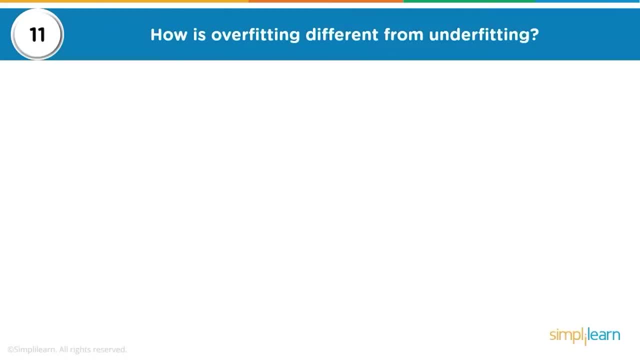 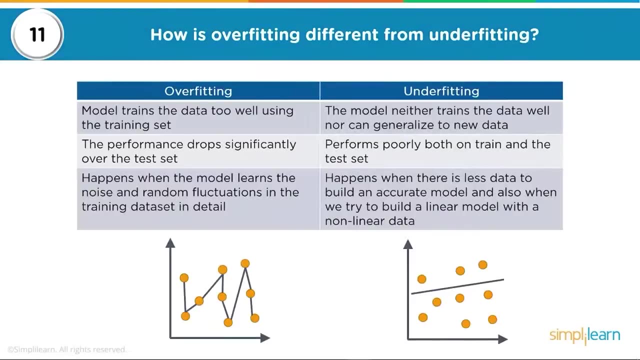 sheet and Oracle table. In data blending, each data source contains its own set of dimensions and measures 11.. How is overfitting different from underfitting? Always a good one? Overfitting Probably the biggest danger in data analytics today. 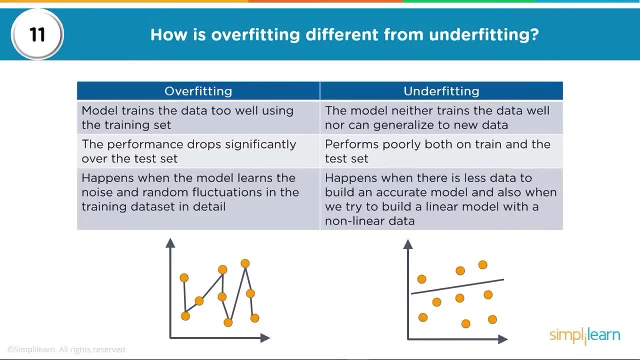 Model trains from the data too well. using the training set, The performance drops significantly over the test set. Happens when the model learns the noise and random fluctuations in the training data set in detail And again the performance drops way below what the test set has. 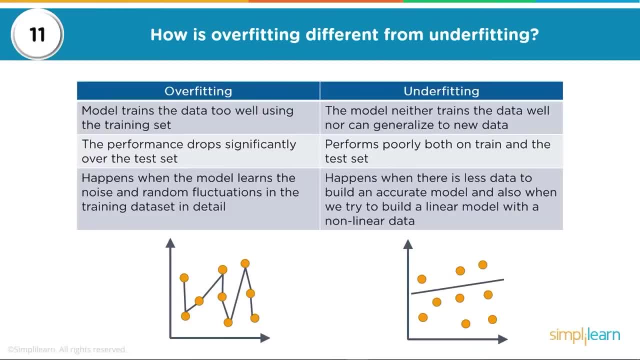 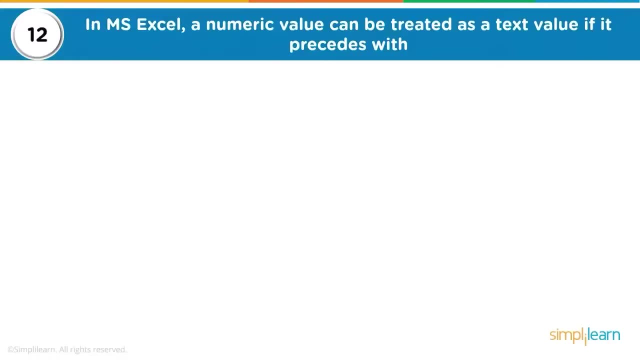 The model neither trains the data well nor can generalize to new data. Performs poorly both on train and the test set. Happens when there is less data to build And also when we try to build a linear model with non-linear data. In Microsoft Excel, a numeric value can be treated as a text value if it proceeds with. 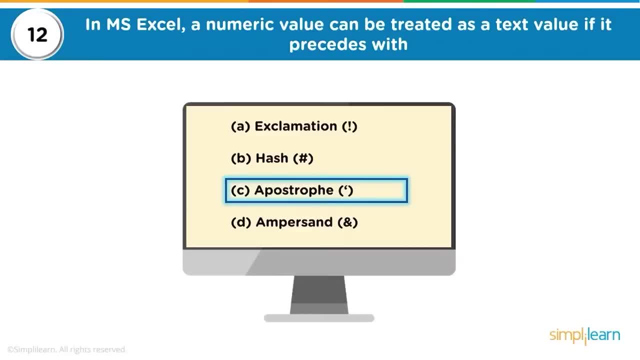 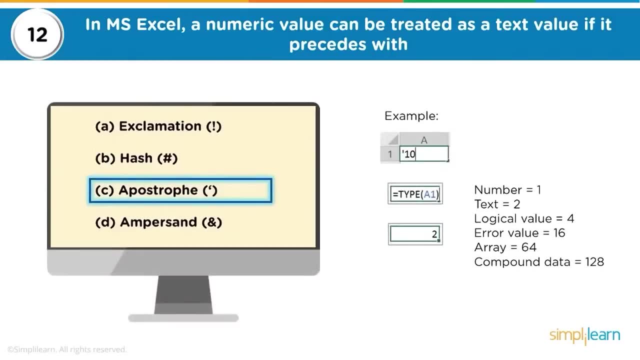 an apostrophe, Definitely not an exclamation. If you're used to programming in Python, you'll look for that hash code and not an amber sign. We can see here: if you enter the value 10 into a fill, but you put the apostrophe in. 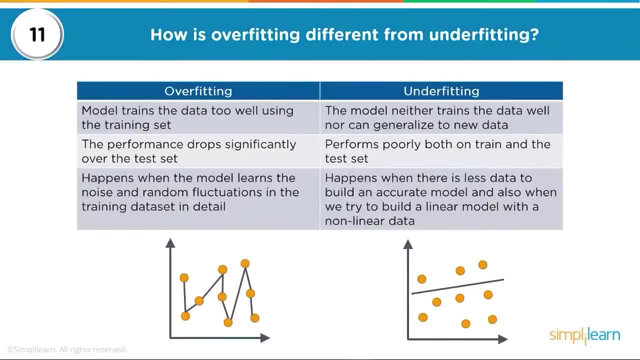 how is overfitting different from underfitting? always a good one. underfitting, always a good one. underfitting, always a good one. overfitting, probably the biggest danger. overfitting, probably the biggest danger. overfitting, probably the biggest danger in data analytics today is overfitting. 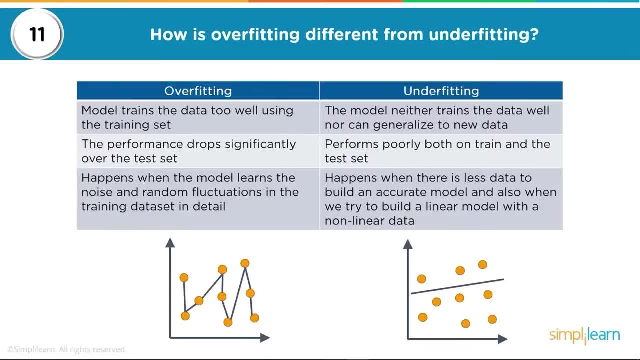 in data analytics today is overfitting. in data analytics today is overfitting. model trains from the data too well. model trains from the data too well. model trains from the data too well. using the training set. using the training set. using the training set, the performance drops significantly over. 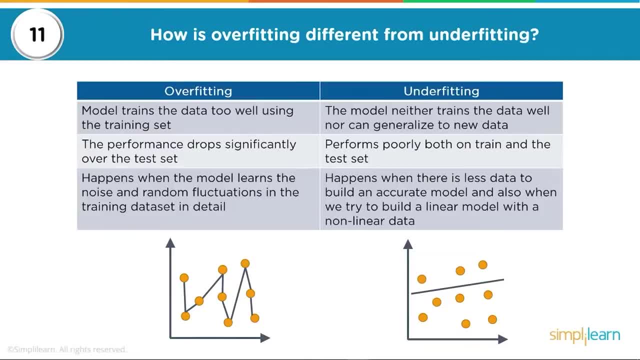 the performance drops significantly over the performance drops significantly over the test set. happens when the model, the test set happens. when the model, the test set happens. when the model learns the noise and random fluctuations. learns the noise and random fluctuations. learns the noise and random fluctuations in the training data set in detail. 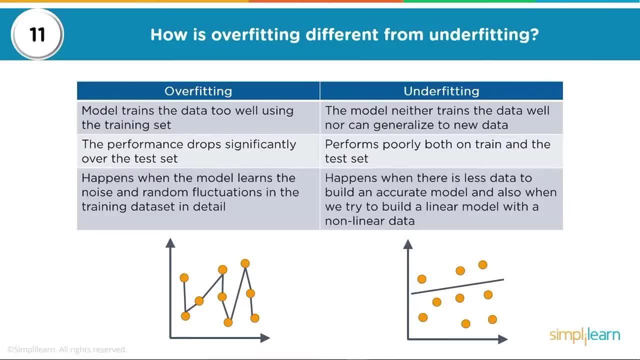 in the training data set in detail, in the training data set in detail. and again the performance drops way and again. the performance drops way and again. the performance drops way below what the test set has, below what the test set has, below what the test set has. the model neither trains the data well. 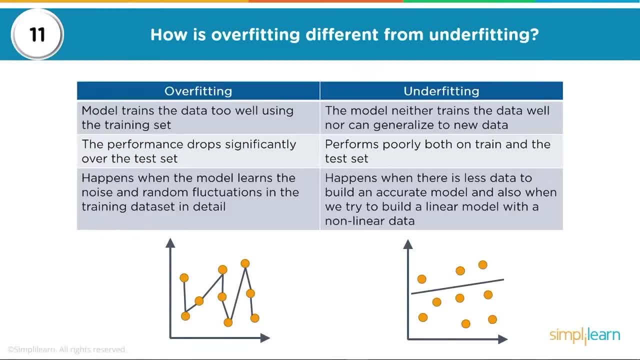 the model neither trains the data well. the model neither trains the data well, nor can generalize to new data, nor can generalize to new data, nor can generalize to new data. performs poorly both on train and the. performs poorly both on train and the. performs poorly both on train and the test set. 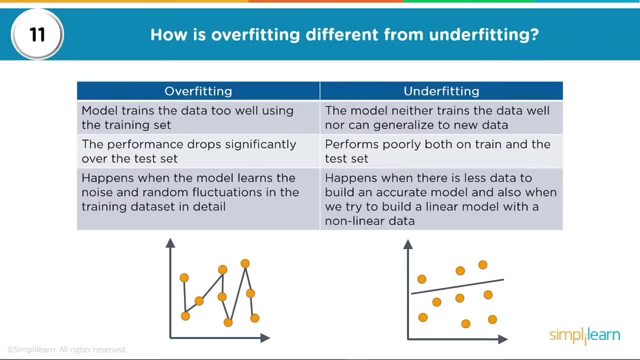 test set. test set happens when there is less data to build. happens when there is less data to build. happens when there is less data to build and an accurate model, and also when we and an accurate model. and also when we and an accurate model, and also when we try to build a linear model with a. 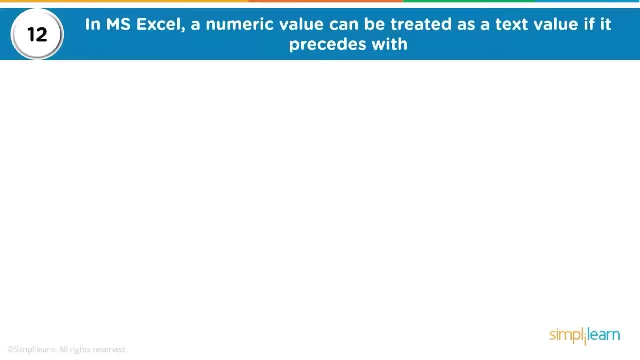 try to build a linear model with a. try to build a linear model with a non-linear data. non-linear data- non-linear data. in microsoft excel. a numeric value can in microsoft excel, a numeric value can in microsoft excel, a numeric value can be treated as a text value if it. 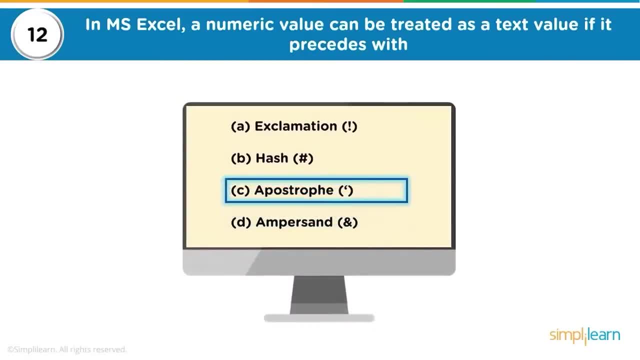 be treated as a text value. if it be treated as a text value, if it proceeds with proceeds, with proceeds, with an apostrophe. definitely not an an apostrophe, definitely not an an apostrophe, definitely not an exclamation, exclamation. exclamation, if you're used to programming in python. 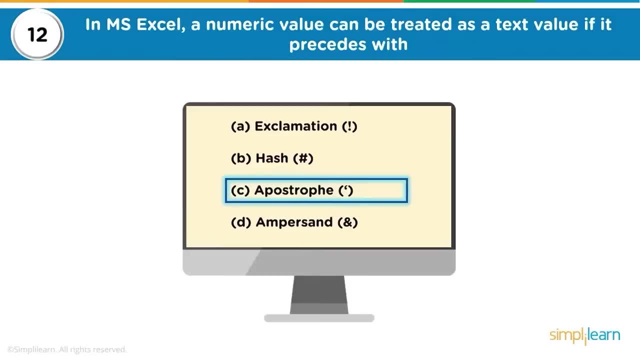 if you're used to programming in python, if you're used to programming in python, you'll look for that hash code. you'll look for that hash code. you'll look for that hash code, and not an amber sign and not an amber sign and not an amber sign. and we can see here, if you enter the 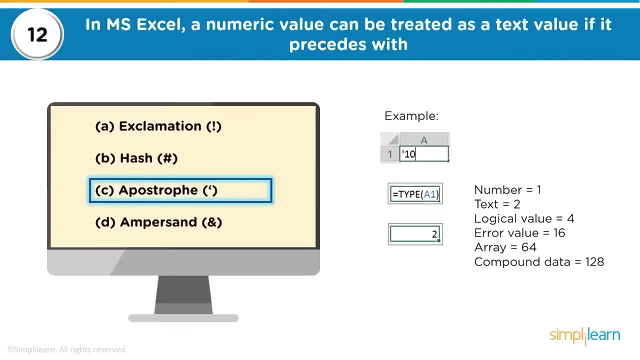 and we can see here if you enter the. and we can see here if you enter the value 10 into a fill, but you put the value 10 into a fill. but you put the value 10 into a fill, but you put the apostrophe in front of it. 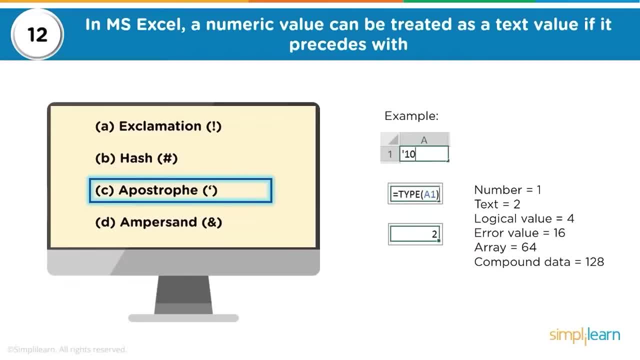 apostrophe in front of it. apostrophe in front of it. it will read that as a text, not as a. it will read that as a text, not as a. it will read that as a text, not as a number. what is the difference between count? what is the difference between count? 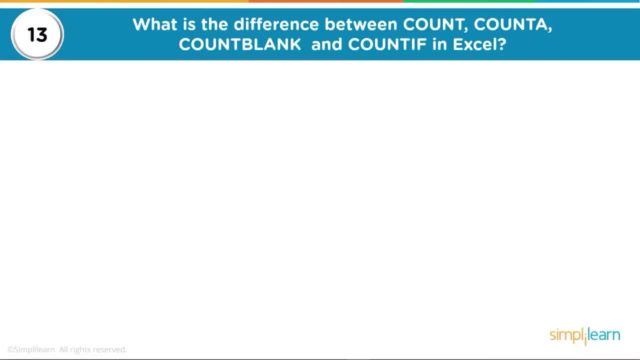 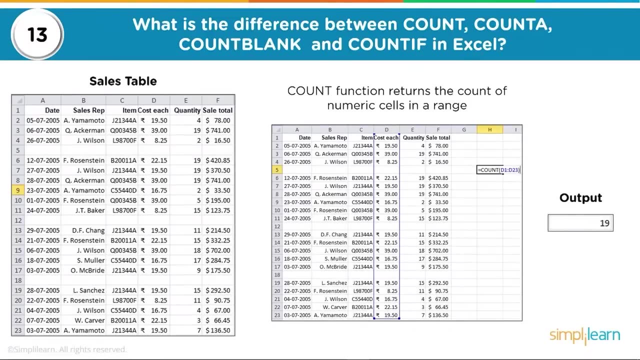 what is the difference between count, count a count blank and count if, count a count blank and count if, count a count blank and count if in excel. we can see here when we run in just. we can see here when we run in just. we can see here when we run in just: count d1 through d23. 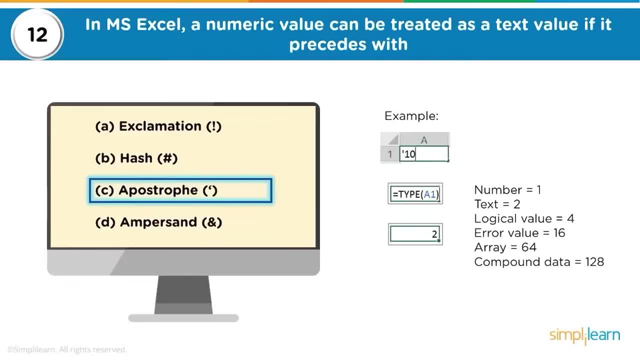 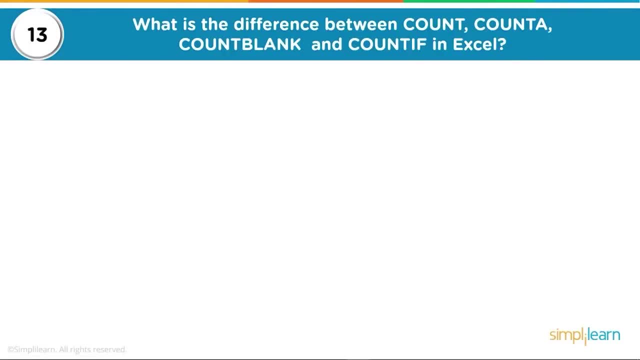 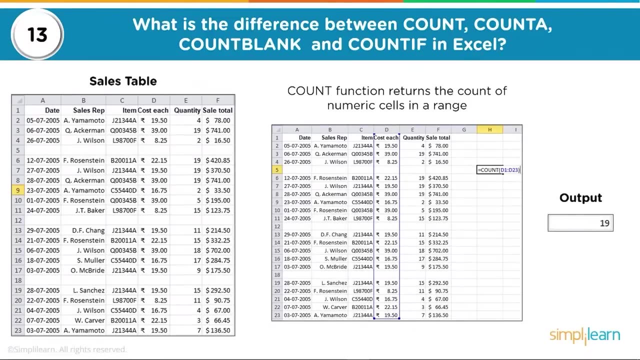 front of it. It will read that as a 10.. Not as a text, not as a number. What is the difference between COUNTA and COUNTIF in Excel? We can see here: when we run in just COUNT D1 through D23, we get 19.. 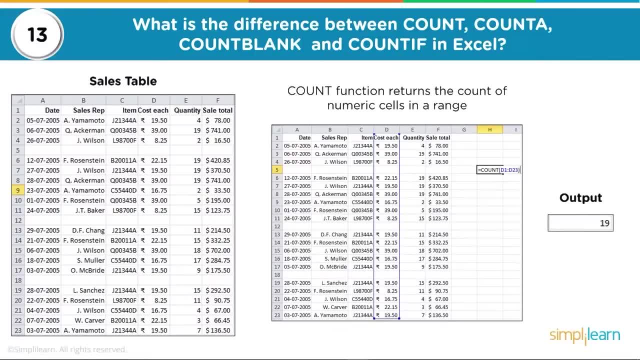 And you'll notice that there is 19 numbers coming down here, And so it doesn't count the cost of each, which is the top bracket, And it doesn't count the blank spaces either. with the straight count, When you do a COUNTA, you'll get the answer as 20.. 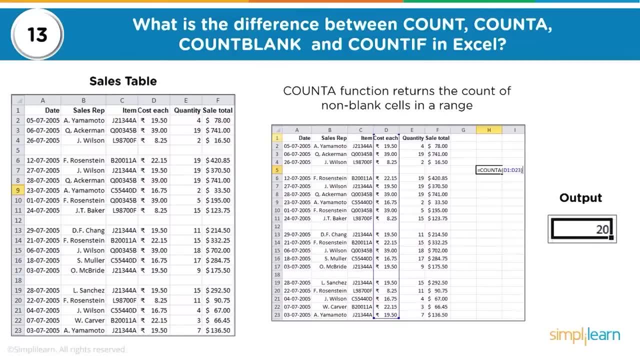 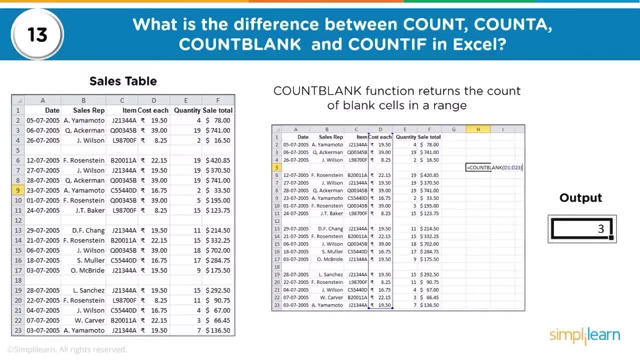 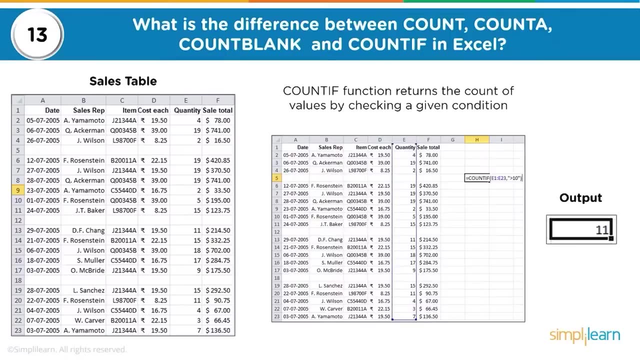 So now when you do COUNTA, it counts all of them, even the title cost of each. When you do COUNTA BLANK, we'll get 3.. Why There's three blank fills? And finally the COUNTIF. If we do COUNTIF of E1 to E23 is greater than 10, there's 11 values in there. 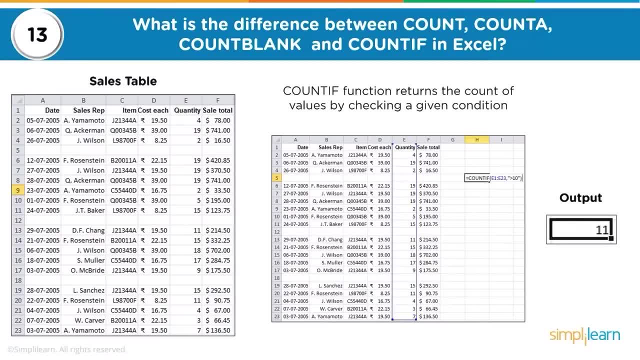 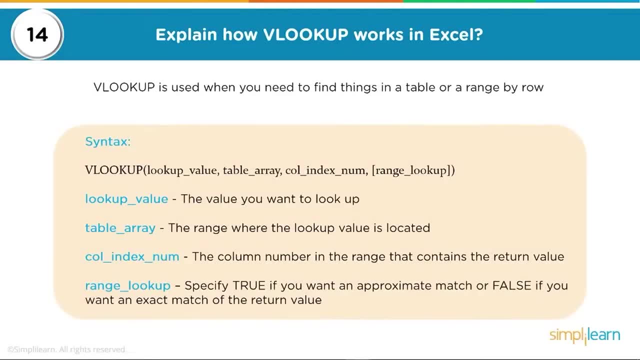 Basic COUNTIF. Basic COUNTIF of whatever's in your column, pretty solid on the table there. Explain how VLOOKUP works in Excel. VLOOKUP is used when you need to find things in a table or a range by row. The syntax has four different parts to it. 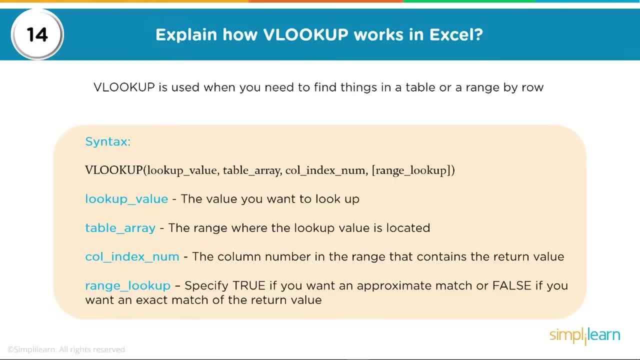 We have our lookup value. that's a value you want to look up. We have our table array. The range where the lookup value is located- Column index number. The column number and range Contains the return value And the range lookup. 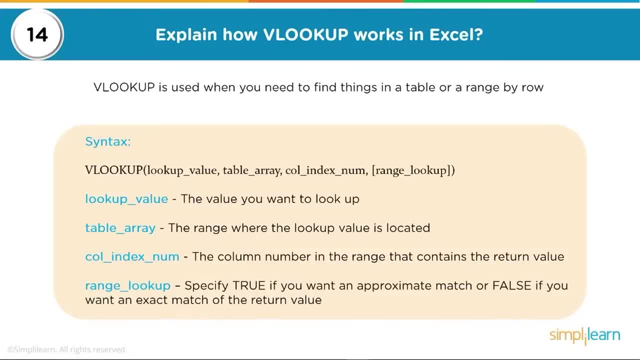 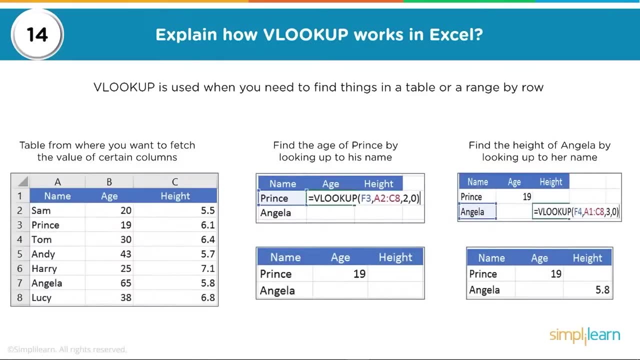 Specify true if you want an approximate match, or false if you want an exact match of the return value. So here we see VLOOKUP F3, A2 to C8, 2 comma 0 for prints. Now they don't show the F3. 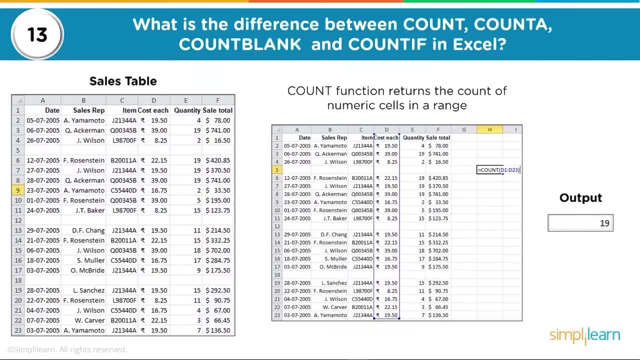 count d1 through d23. count d1 through d23: we get 19, and you'll notice that there we get 19 and you'll notice that there we get 19, and you'll notice that there is 19 is 19, is 19 numbers coming down here, and so it. 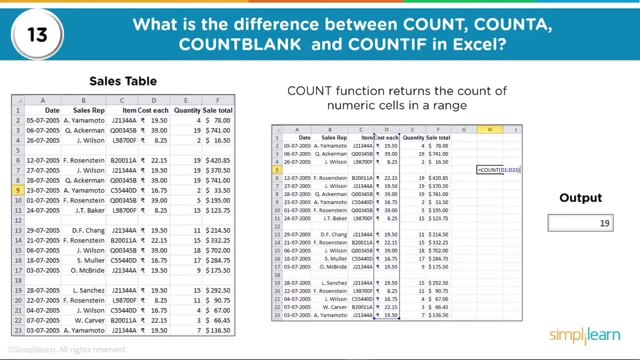 numbers coming down here, and so it numbers coming down here, and so it doesn't count. the cost of each doesn't count. the cost of each doesn't count. the cost of each, which is a top bracket, it doesn't count. which is a top bracket, it doesn't count. 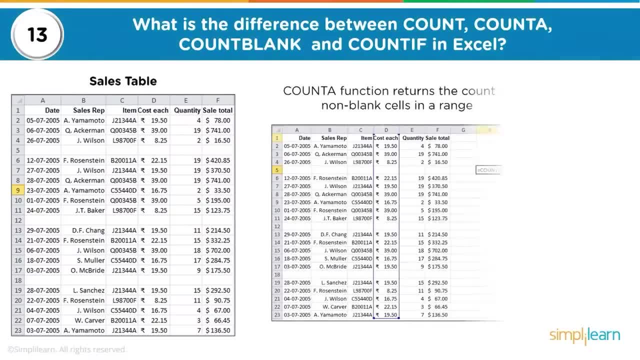 which is a top bracket. it doesn't count the blank spaces. either the blank spaces, either the blank spaces, either with the straight count. when you do a with the straight count, when you do a with the straight count, when you do a count, count, count a. you'll get the answer is 20. so now when 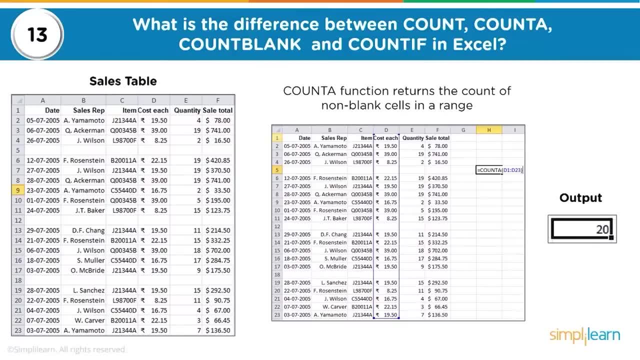 a, you'll get. the answer is 20. so now when a, you'll get the answer is 20. so now, when you do count a, it counts all of them. you do count a, it counts all of them. you do count a, it counts all of them, even the title, cost of each. 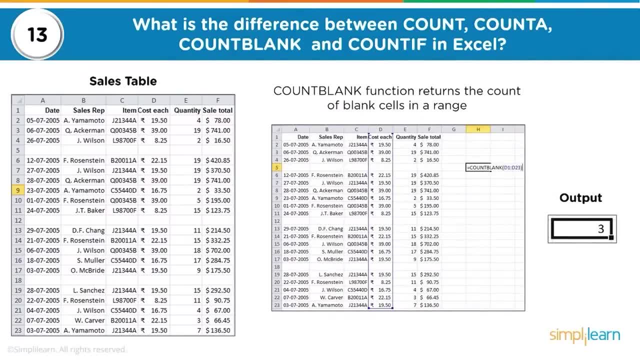 even the title cost of each. even the title cost of each. when you do count blank, we'll get three. when you do count blank, we'll get three. when you do count blank, we'll get three. why there's three blank fields? why there's three blank fields? 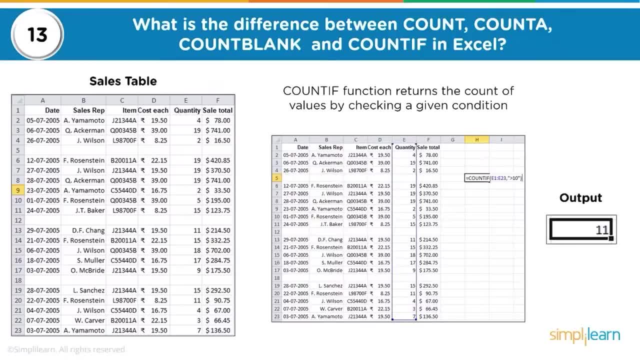 why there's three blank fields. and finally the count if. if we do count. and finally the count if. if we do count. and finally the count if. if we do count. if of e, if of e, if of e, 1 to e, 23 is greater than 10, there's 11. 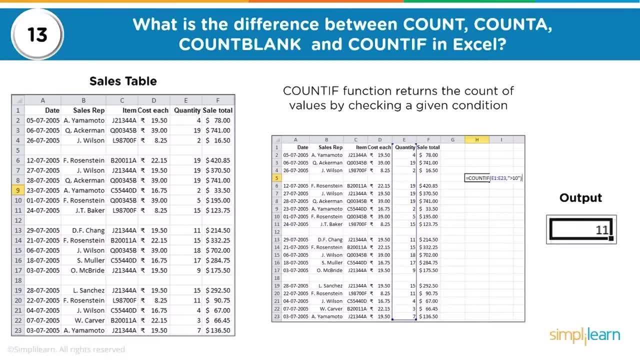 1 to e 23 is greater than 10. there's 11: 1 to e 23 is greater than 10. there's 11 values in there. basic counting of values in there. basic counting of values in there. basic counting of whatever's in your column, pretty solid on. 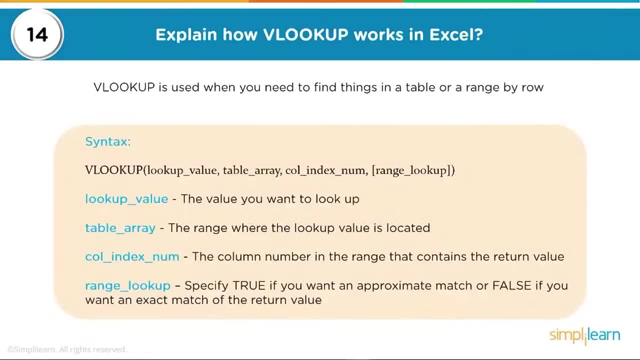 whatever's in your column pretty solid on whatever's in your column pretty solid on the table there, the table there, the table there. explain how vlookup works in excel. explain how vlookup works in excel. explain how vlookup works in excel. vlookup is used when you need to find. 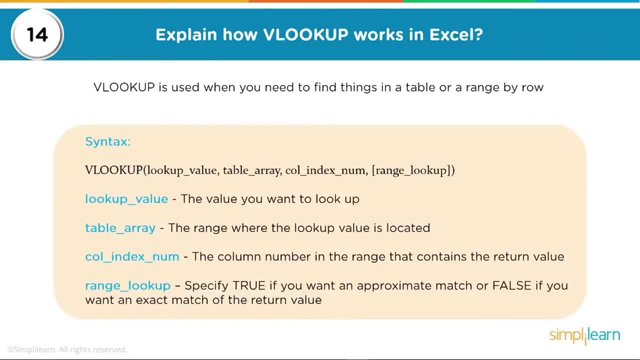 vlookup is used when you need to find. vlookup is used when you need to find things in a table or a range by row. things in a table or a range by row. things in a table or a range by row. the syntax has four different parts to: 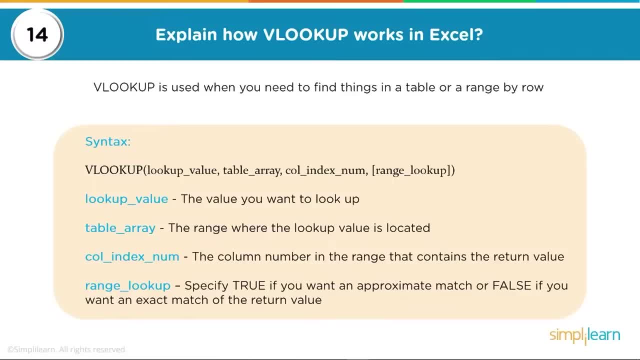 the syntax has four different parts to the syntax has four different parts to it it it. we have our lookup value. that's a value. we have our lookup value. that's a value. we have our lookup value. that's a value you want to look up. we have our table. 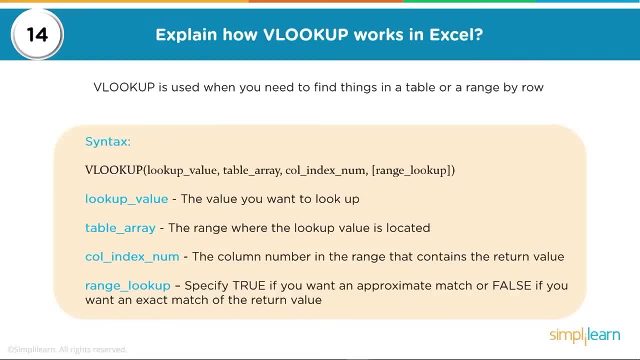 you want to look up? we have our table. you want to look up? we have our table array, array, array: the range where the lookup value is: the range where the lookup value is. the range where the lookup value is located, located, located. column index number: the column number. 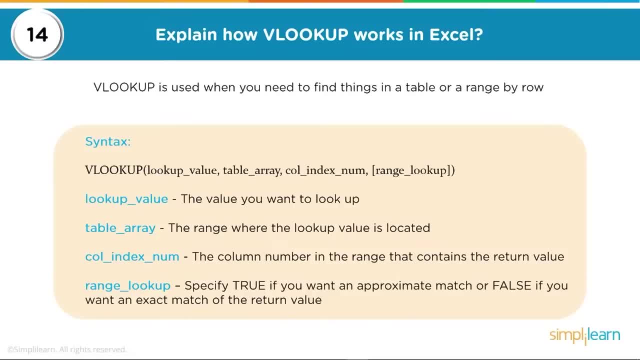 column index number. the column number. column index number. the column number and range that contains the return and range. that contains the return and range. that contains the return value. value, value and the range lookup. specify true if. and the range lookup specify true if. and the range lookup specify true if you want an approximate match, or false if. 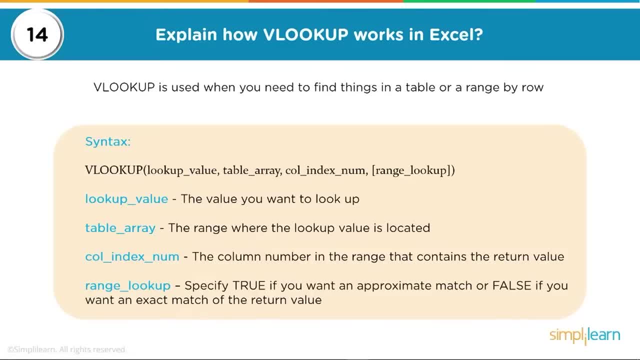 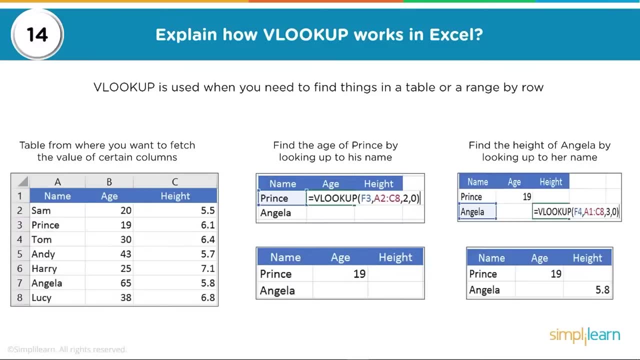 you want an approximate match or false? if you want an approximate match or false. if you want an exact match of the return, you want an exact match of the return. you want an exact match of the return. they don't show the f3. f3 is the actual. they don't show the f3. f3 is the actual. they don't show the f3. f3 is the actual cell that prints is in. that's what we're cell that prints is in. that's what we're cell that prints is in. that's what we're looking at is f3. so there's your prince. 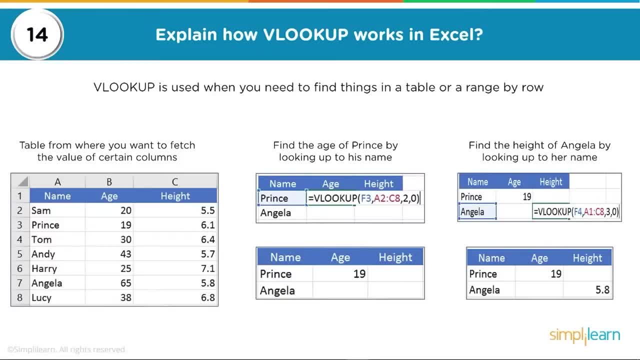 looking at is f3, so there's your prince looking at is f3, so there's your prince. he pulls in from f3. he pulls in from f3. he pulls in from f3. a2 to c8: is the the data we're looking? a2 to c8: is the the data we're looking? 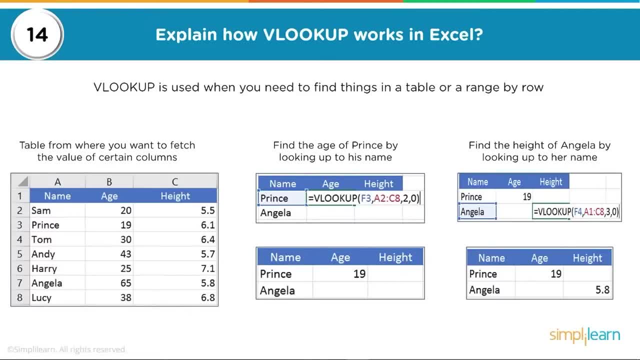 a2 to c8 is the the data we're looking into, and then number two is a column in into and then number two is a column in into and then number two is a column in that data. so in this case we're looking that data. so in this case we're looking. 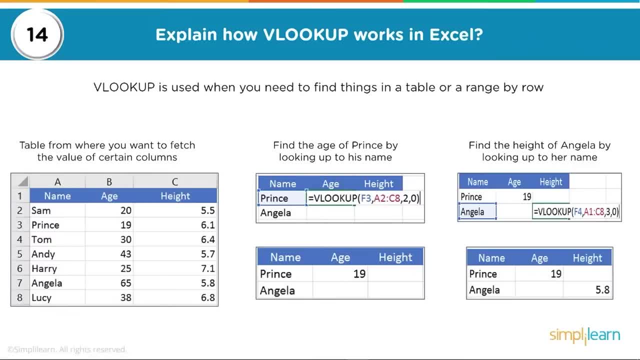 that data. so in this case we're looking for for for age and we count. name is one. age is two. age and we count name is one. age is two. age and we count name is one, age is two. keep in mind: this is excel versus a lot. 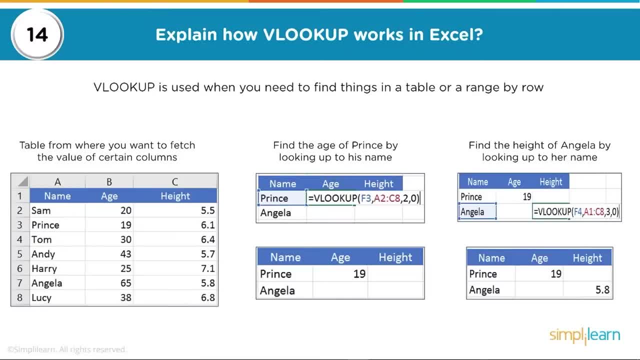 keep in mind: this is excel versus a lot. keep in mind this is excel versus a lot of your, of your, of your. python and programming languages is python and programming languages is python and programming languages is where you start at zero. where you start at zero, where you start at zero in excel, we always look at the cells as: 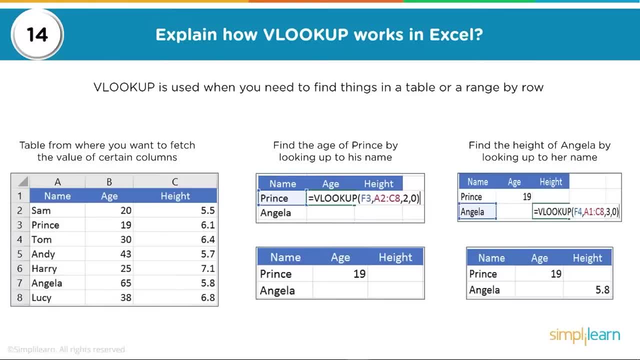 in excel, we always look at the cells. as in excel, we always look at the cells as one, two, three, so two represents the age. one, two, three so two represents the age. one, two, three so two represents the age. zero is zero is zero is false for having an exact matchup versus: 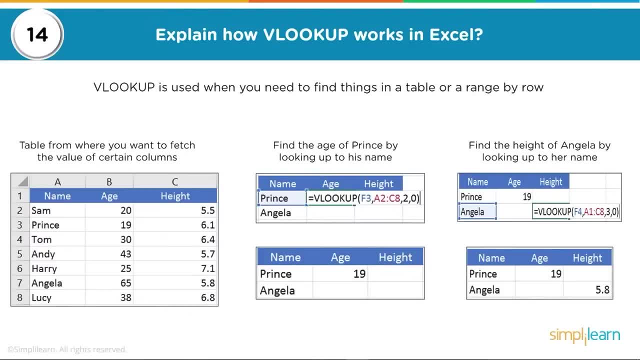 false for having an exact matchup versus false for having an exact matchup versus one. we don't actually need to worry about one. we don't actually need to worry about one. we don't actually need to worry about that too much in this. that too much in this. 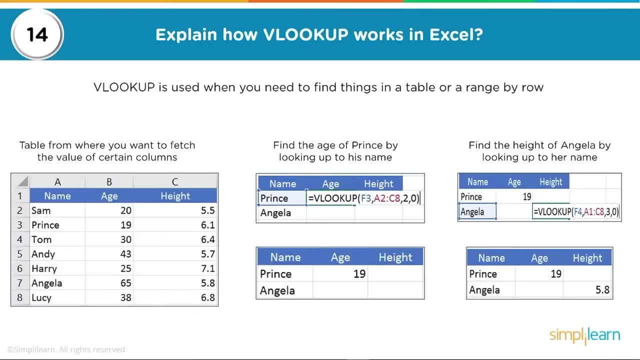 that too much in this zero. or one would work with this example zero, or one would work with this example zero, or one would work with this example, and you can see with the angela lookup, and you can see with the angela lookup and you can see with the angela lookup again, her name would be in the f column. 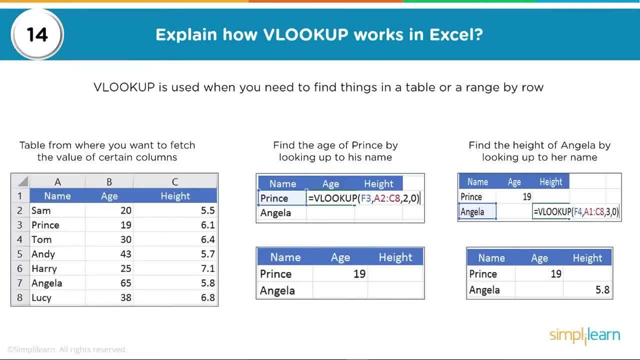 again, her name would be in the f column. again, her name would be in the f column number four. that's what the f4 stands. number four, that's what the f4 stands. number four- that's what the f4 stands for- is where they pulled angela from. 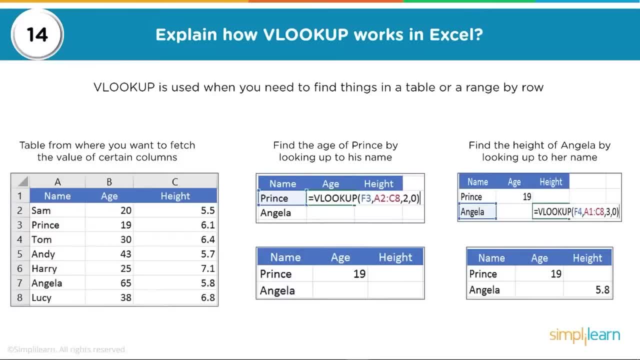 F3 is the actual cell that prints is in. That's what we're looking at is F3.. So there's your prints. He pulls in from F3.. A2 to C8.. F3 is the data we're looking into. 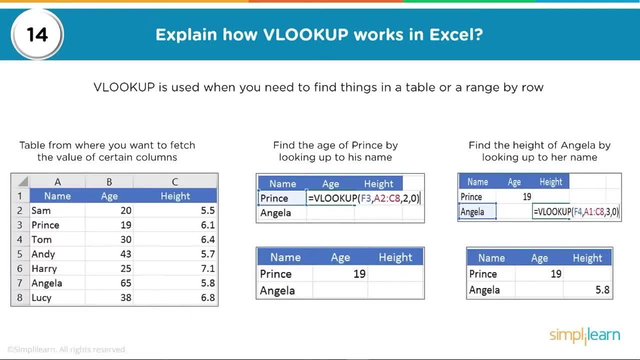 And then number 2 is a column in that data. So in this case we're looking for age And we count name as 1, age as 2.. Keep in mind, this is Excel versus a lot of your Python and programming languages, where 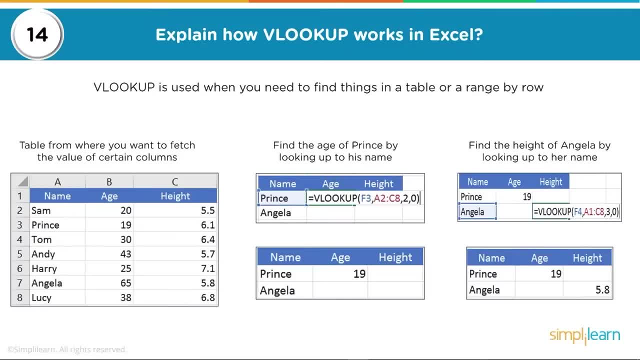 you start at 0.. In Excel, we always look at the cells as 1,, 2, 3.. So 2 represents the age. 0 is false for having an exact matchup. 0 is false for having an exact matchup. 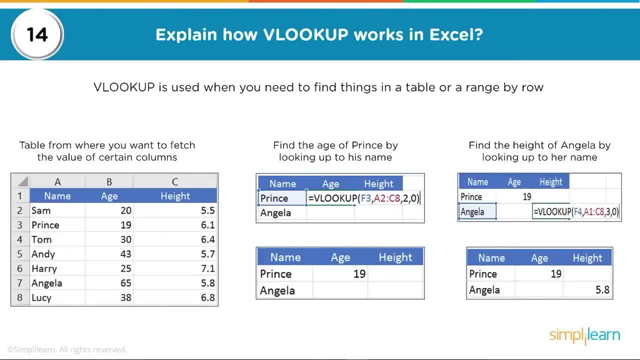 Versus 1.. We don't actually need to worry about that too much in this. 0 or 1 would work with this example And you can see with the Angela lookup again. her name would be in the F column number 4.. 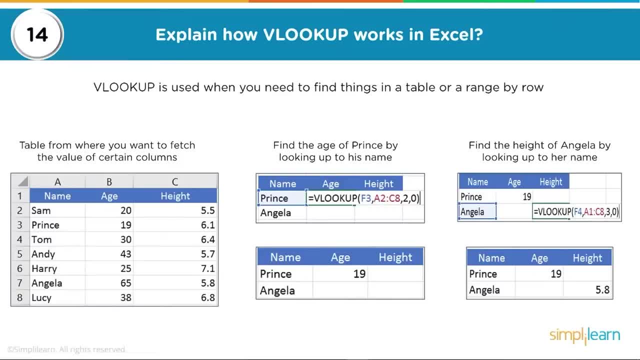 That's what the F4 stands for is where they pulled Angela from. And then you have A1 to C8. And then we're looking at number 3.. So number 3 is height, Name being 1,, age 2, and then height 3.. 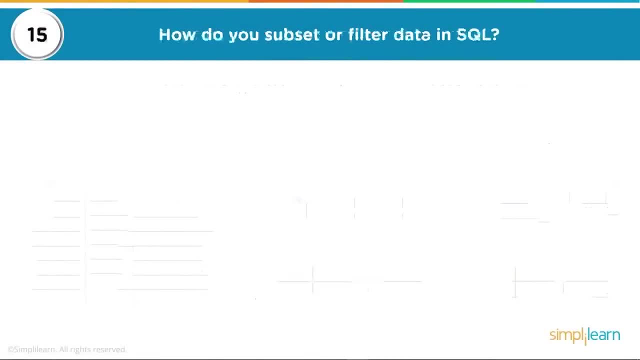 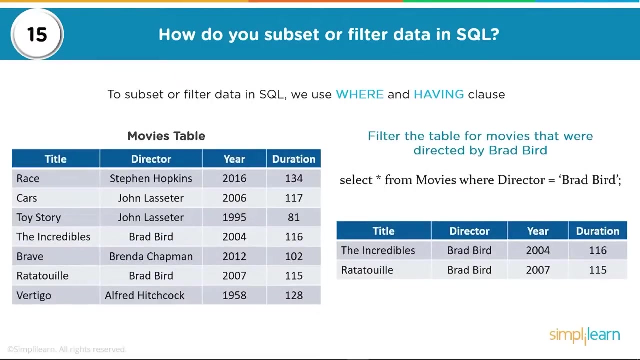 And you'll see here: pulls in her height 5.8.. So we're going to run Jump over to SQL. How do you subset or filter data in SQL? To subset or filter data in SQL, we use WHERE and HAVING clause. 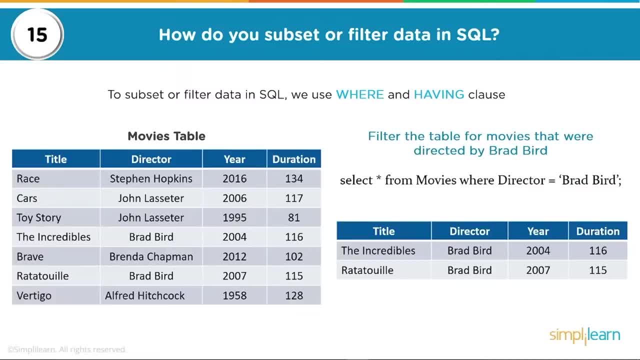 You can see, we have a nice table on the left where we have the title, the director, the year, the duration. We want to filter the table for movies that were directed by Brad Bird. Why? Just because we want to know what Brad Bird did. 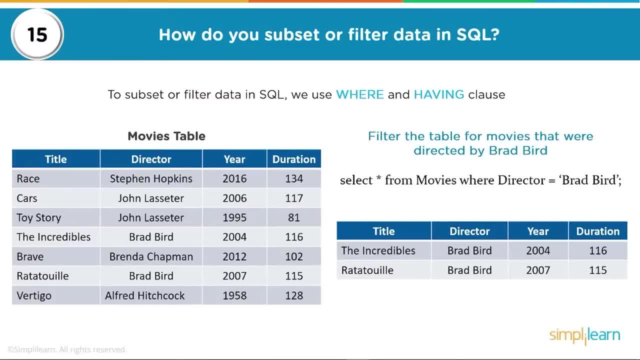 So we're going to do SELECT STAR. You should know that the star refers to All. In this case, what are we going to return? We're going to return all: title, directory, year and duration. That's what you mean by all. 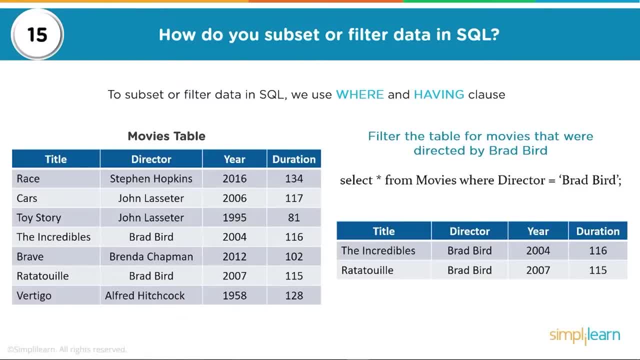 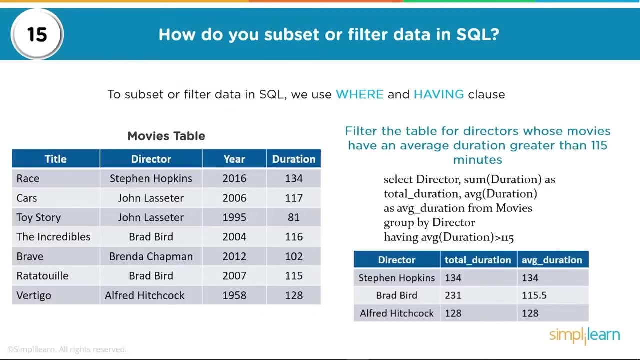 From movies. Movies being our table. WHERE director equals Brad Bird And you can see he comes back and he did the incredible on Ratatouille. To subset or filter data SQL, we can also use the WHERE and HAVING clause, So we're going to take a closer look at the different ways we can filter here. 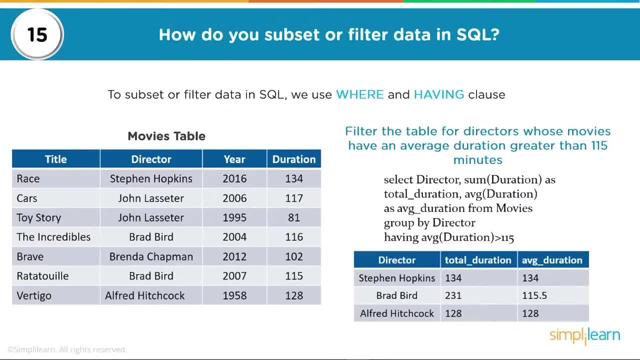 Filter the table for directors whose movies have an average value Average duration greater than 115 minutes. So there's a lot of really cool things into this SQL query And these SQL queries can get pretty crazy. Select director: sum duration as total duration. average duration as average duration. 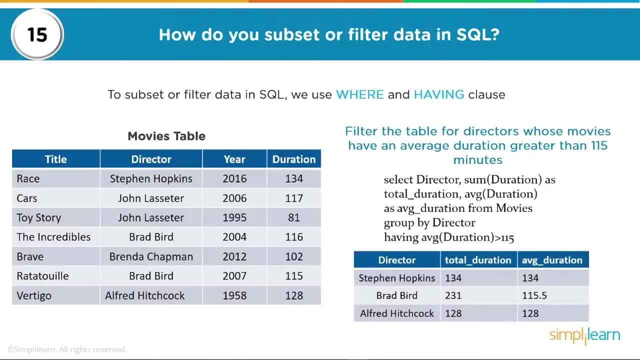 From movies Group by director, having average duration greater than 115.. So again, what are we going to return? We're going to return whatever we put in our select, Which, in this case, is director. We're going to have total duration and that's going to be the sum of the duration. for is where they pulled angela from, for is where they pulled angela from. and then you have a1 to c8, and then, and then you have a1 to c8, and then, and then you have a1 to c8, and then we're looking at. 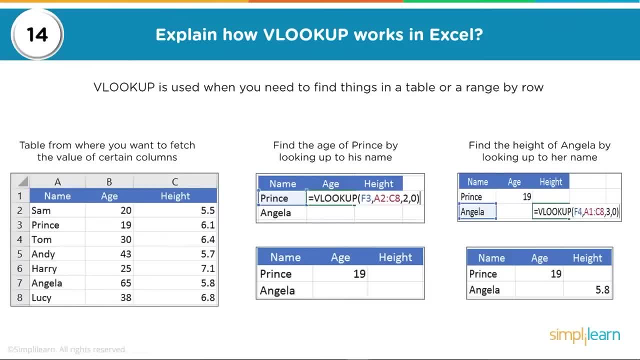 we're looking at. we're looking at number three. so number three is height number three. so number three is height number three. so number three is height, name being one h2 and then height three, name being one, h2 and then height three, name being one, h2 and then height three, and you'll see here pulls in her height. 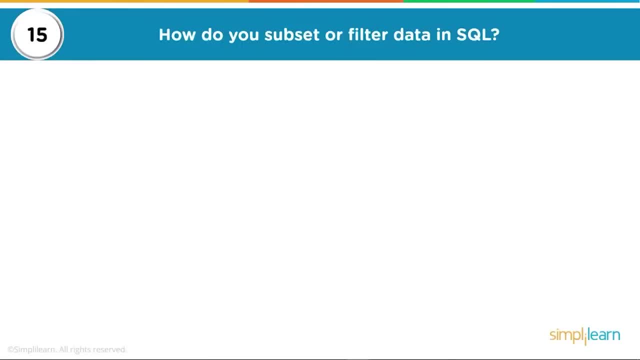 and you'll see here: pulls in her height. and you'll see here: pulls in her height: 5.8, 5.8, 5.8. so we're going to run jump over to sql. so we're going to run jump over to sql. so we're going to run, jump over to sql. how do you subset or filter data in sql? 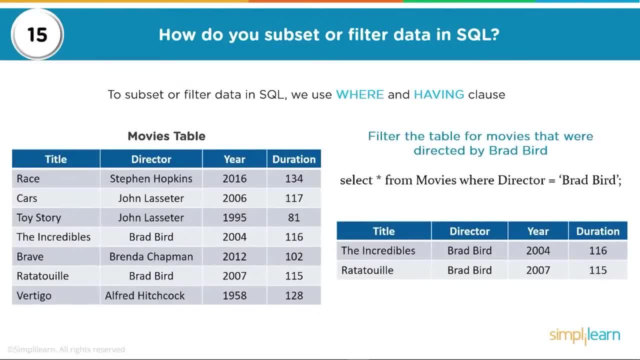 how do you subset or filter data in sql. how do you subset or filter data in sql. to subset or filter data in sql. we use to subset or filter data in sql. we use to subset or filter data in sql. we use where and having clause: where and having clause. 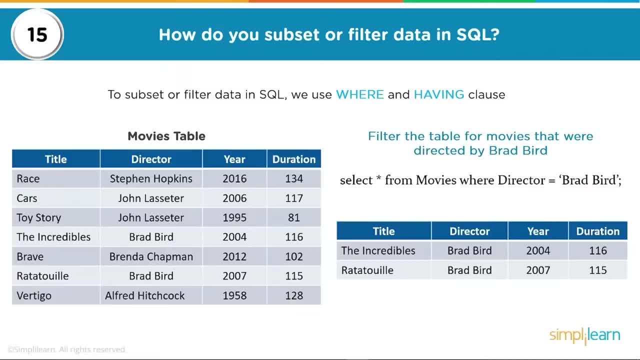 where and having clause. you can see we have a nice table on the. you can see we have a nice table on the. you can see we have a nice table on the left, where we have the title left, where we have the title left, where we have the title, the director, the year, the duration. 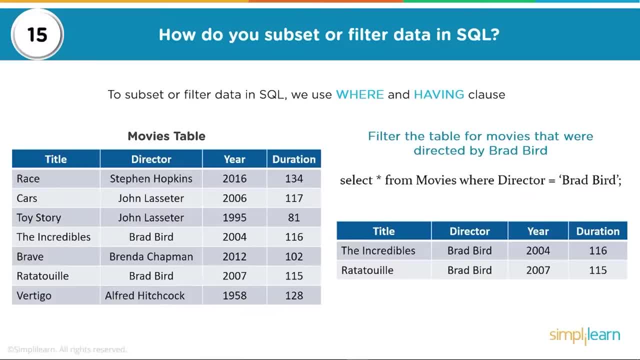 the director: the year, the duration. the director: the year, the duration. we want to filter the table for movies. we want to filter the table for movies. we want to filter the table for movies that were directed by, that were directed by, that were directed by brad bird. why? just because we want to know. 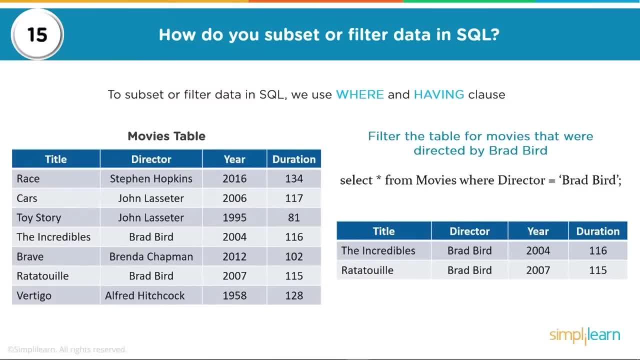 brad bird. why? just because we want to know brad bird. why? just because we want to know what brad bird did, what brad bird did, what brad bird did. so we're going to do select star you. so we're going to do select star you. 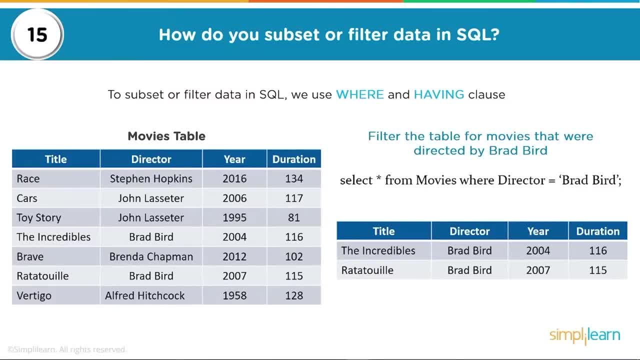 so we're going to do select star. you should know that the star refers to. should know that the star refers to. should know that the star refers to all in this case. where. what are we going to all in this case? where? what are we going to all in this case? where? what are we going to return? we're going to return. 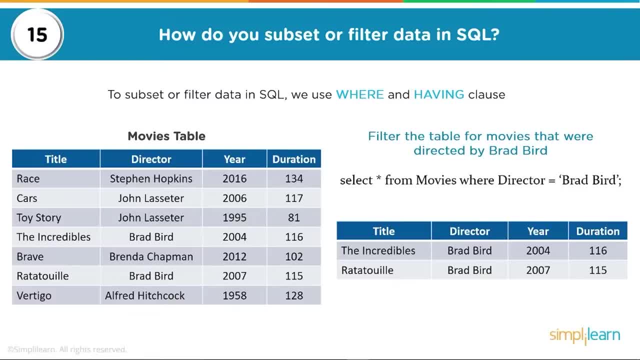 return. we're going to return, return. we're going to return all title directory year and duration. all title directory year and duration. all title directory year and duration. that's what you mean by all. that's what you mean by all. that's what you mean by all from movies, movies being our table. 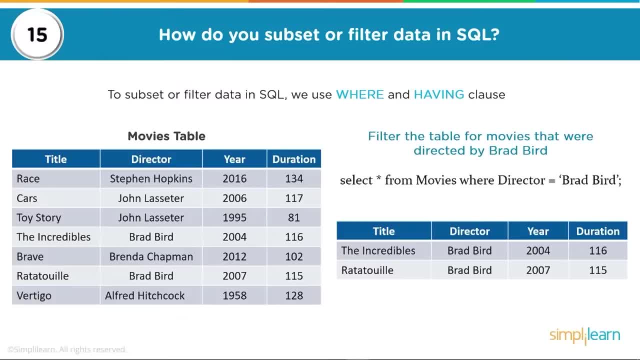 from movies, movies being our table, from movies, movies being our table, where director equals brad bird and you, where director equals brad bird and you, where director equals brad bird and you can see, can see, can see. he comes back and he did the incredible. he comes back and he did the incredible. 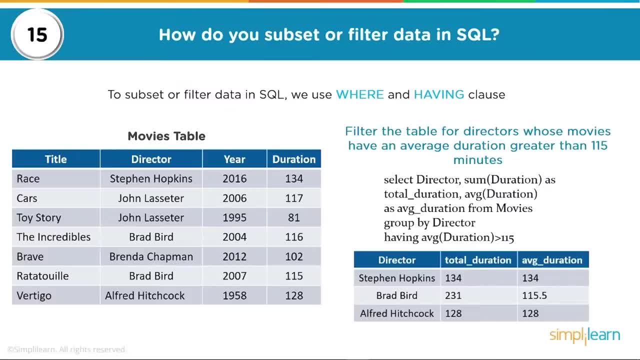 he comes back and he did the incredible and ratatouille and ratatouille and ratatouille. to subset or filter data sql: we can also to subset or filter data sql. we can also to subset or filter data sql. we can also use the. 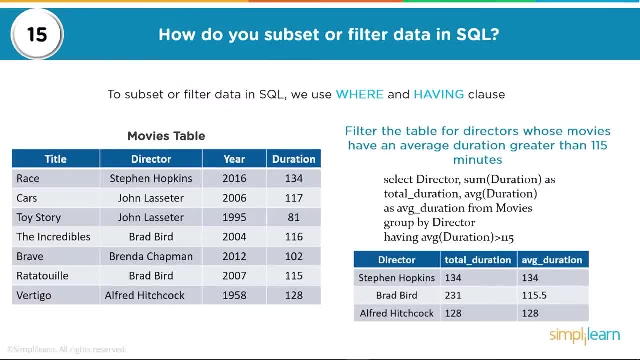 use the use, the where and having clause. so we're going to where and having clause. so we're going to where and having clause. so we're going to take a closer look at the take a closer look at the take a closer look at the different ways we can filter it here. 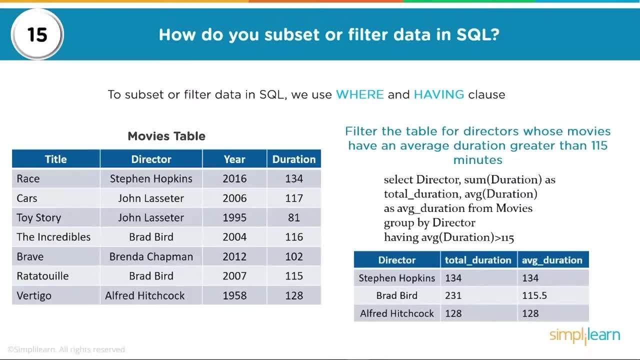 different ways we can filter it here. different ways we can filter it here: filter the table for directors whose filter. the table for directors whose filter. the table for directors whose movies have an average duration. greater movies have an average duration. greater movies have an average duration greater than 115. 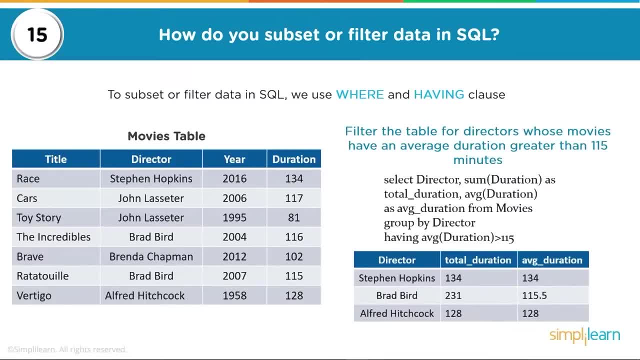 than 115, than 115 minutes. so there's a lot of really cool minutes. so there's a lot of really cool minutes. so there's a lot of really cool things into this sql things, into this sql things, into this sql query and these sql queries can get. 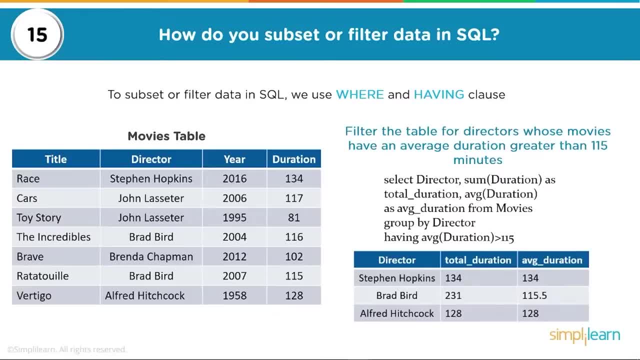 query and these sql queries can get query and these sql queries can get pretty crazy, pretty crazy, pretty crazy. select director. some duration as total select director. some duration as total select director. some duration as total duration. average duration as average duration. average duration as average duration. average duration as average duration from movies. group by director. 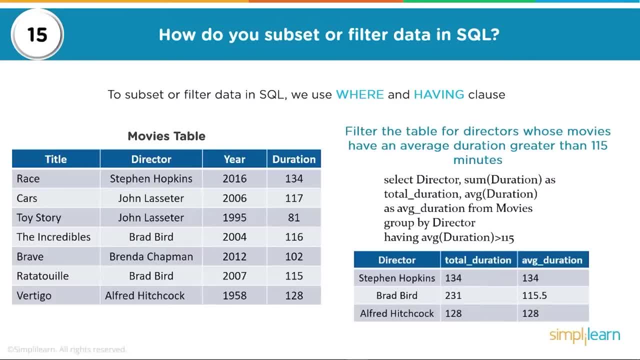 duration from movies group by director. duration from movies group by director having average duration greater than 115. having average duration greater than 115. having average duration greater than 115. uh, so again, what are we going to return? uh, so again, what are we going to return? 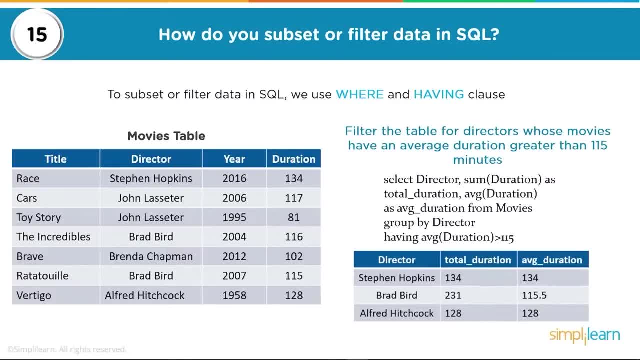 uh. so again, what are we going to return? we're going to return whatever we put in. we're going to return whatever we put in. we're going to return whatever we put in our select, which, in this case, is our select, which, in this case, is our select, which, in this case, is director. we're going to have total. 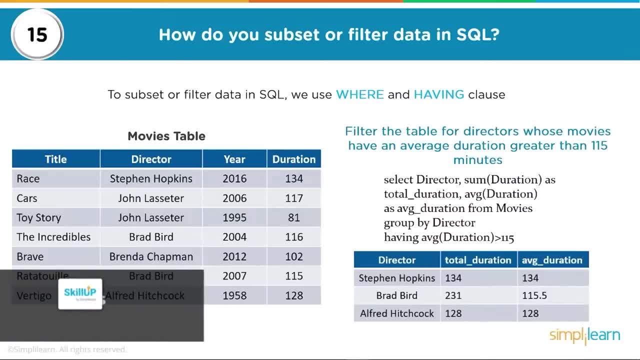 director. we're going to have total director. we're going to have total duration and that's going to be the sum duration and that's going to be the sum duration and that's going to be the sum of the duration. we're going to have the of the duration we're going to have the. 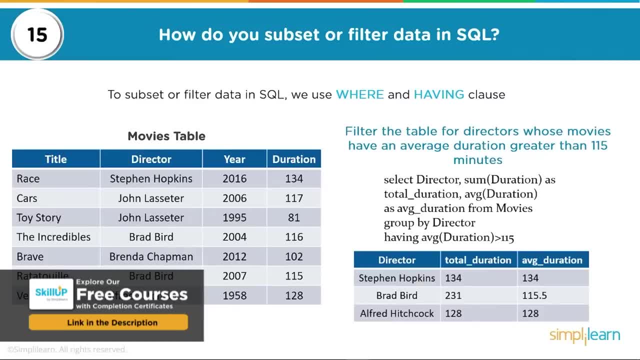 We're going to have the average duration, average underscore duration, which is going to be the average duration on there, And then we of course go ahead and group by director- And we want to make sure we group them by anyone that has an having an average duration greater than 115. 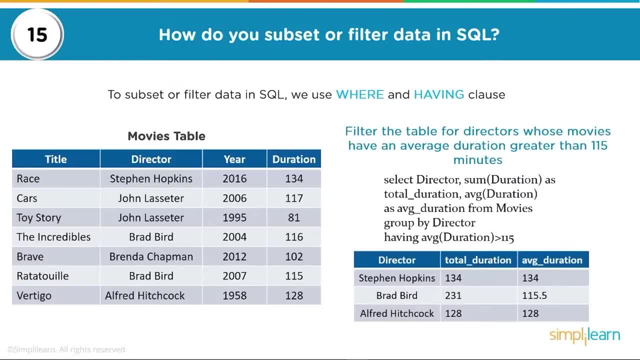 These SQL queries are so important- I don't know how many times the SQL comes up- and there's so many different other languages, not just MySQL and not Microsoft SQL, but in addition to that where the SQL language comes in, especially with Hadoop and other areas. 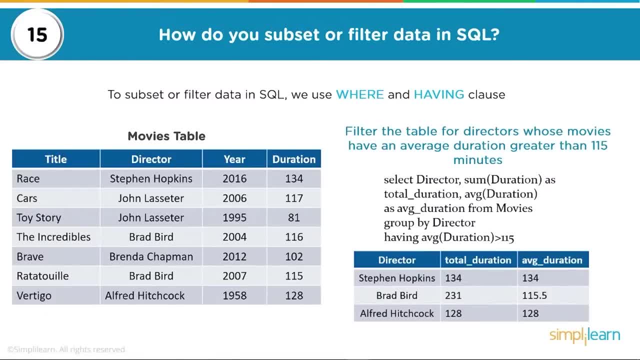 So you really should know your basic SQL. It doesn't hurt to get that little cheat sheet and glance over it and double-check some of the different features in SQL. What is the difference between where and having clause in SQL Where? Where clause works. 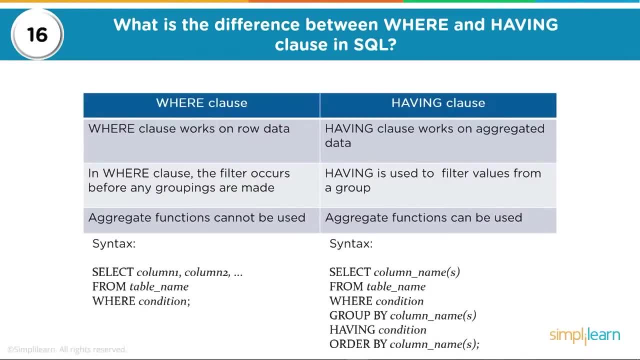 It works on row data In where clause the filter- occurs before any groupings are made. Aggregate functions cannot be used, So the syntax is: select your columns from table where what the condition is Having clause works on aggregated data. Having is used to filter values from a group. 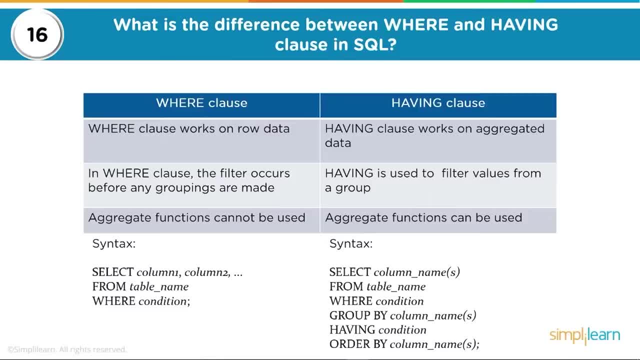 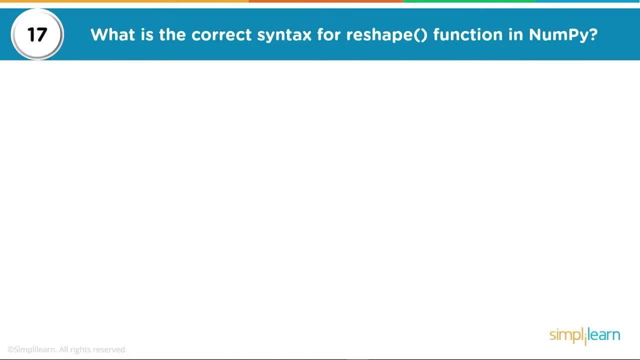 Aggregate functions can be used And the syntax is: select column names from table where the condition is Grouped by having a condition ordered by column names. What is the correct syntax for reshape function in NumPy? So we're going to jump to the NumPy array program. 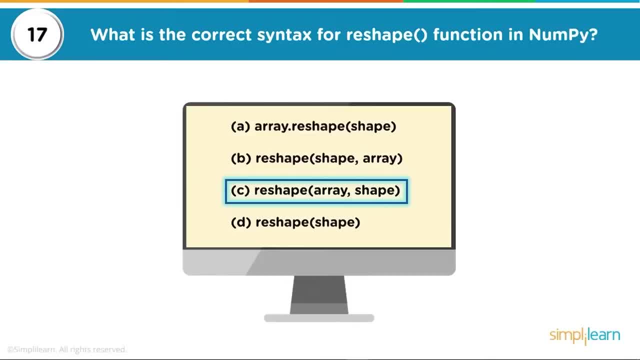 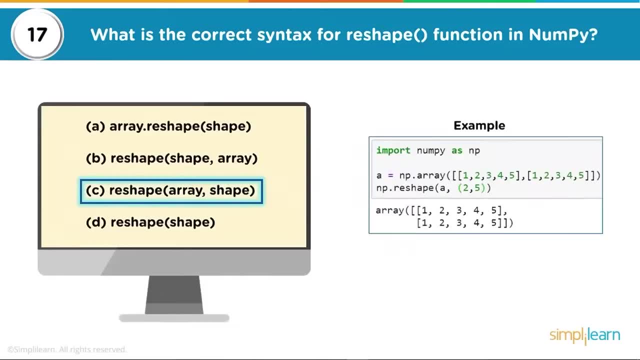 And what you come up with is you have- in this case it would be NumPyreshape. A lot of times you do an import. NumPy is in P, Reshape, and then your array and the new shape. And you can see here as the actual example comes in, the reshape is A. 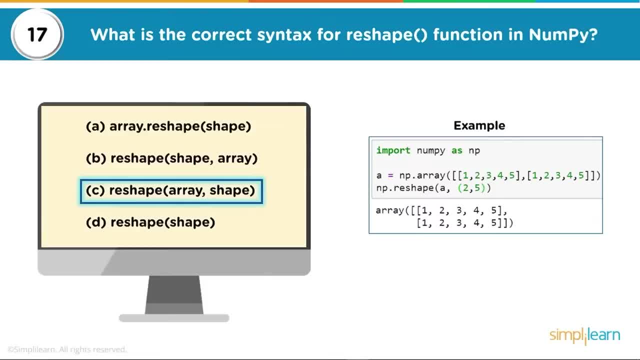 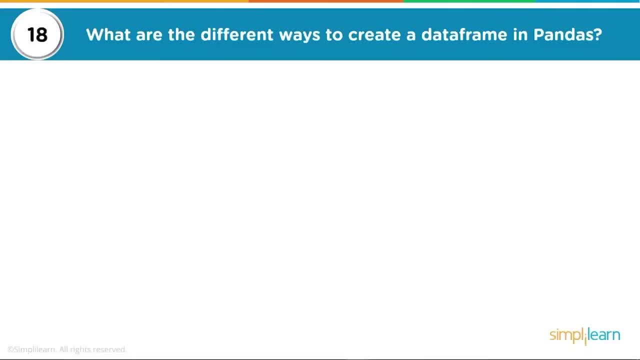 And we're going to reshape it in 2, 5 setups And you can see the printout in there that prints in two rows with five values in each one. What are the different ways to create a data frame in Pandas? Well, we can do it by initializing a list. 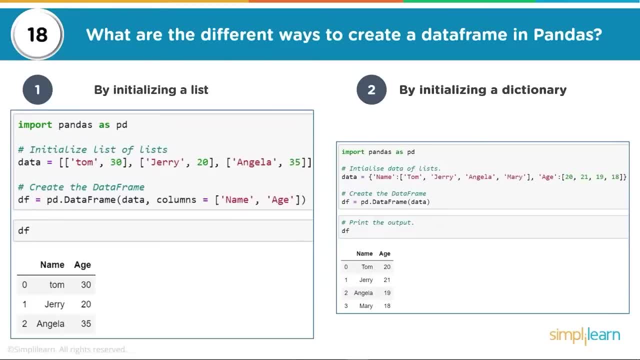 So you can port your Pandas as PD. Very common Data equals Tom 30,, Jerry 20,, Angela 35. We'll go ahead and create the data frame And we'll say PDdataFrame is the data Columns equals. 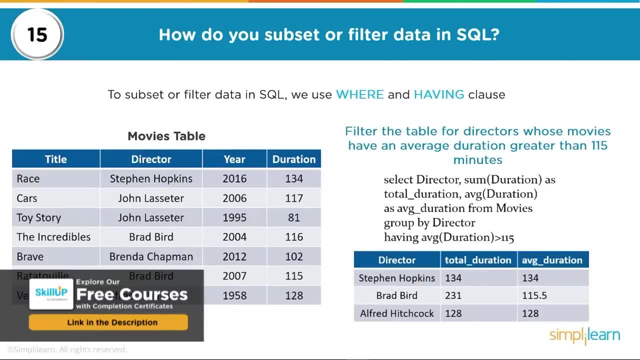 of the duration we're going to have the average duration. average underscore- average duration- average underscore- average duration- average underscore duration, which is going to be the average duration, which is going to be the average duration, which is going to be the average duration on there. duration on there. 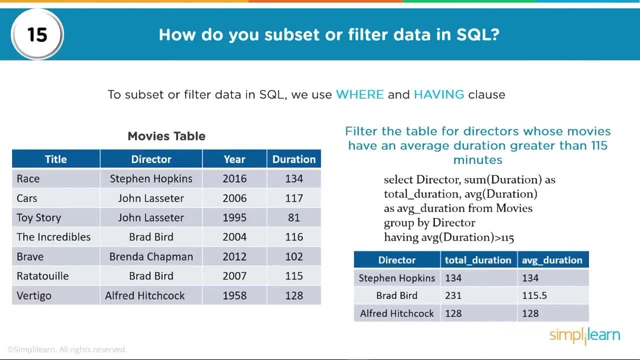 duration on there. and then we of course go ahead and group, and then we of course go ahead and group, and then we of course go ahead and group by director and we want to make sure we by director and we want to make sure we by director and we want to make sure we group them by. 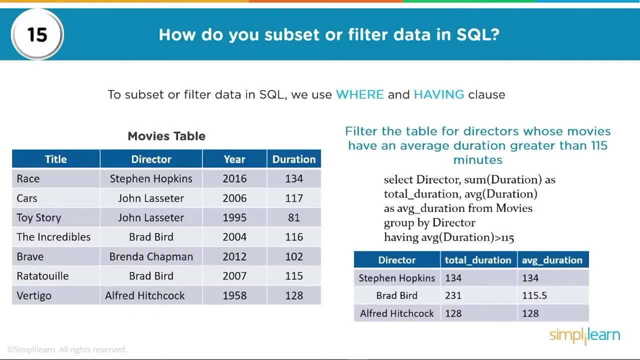 group them by. group them by anyone that has an having an average. anyone that has an having an average. anyone that has an having an average duration greater than 115.. duration greater than 115.. duration greater than 115.. these sql queries are so important. 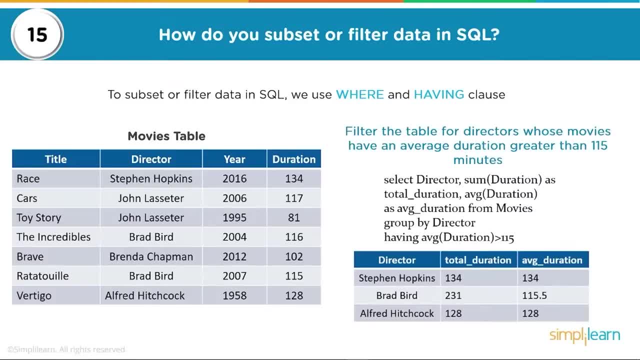 these sql queries are so important. these sql queries are so important. i don't know how many times your the sql. i don't know how many times your the sql. i don't know how many times your the sql comes up and there's so many different comes up and there's so many different. 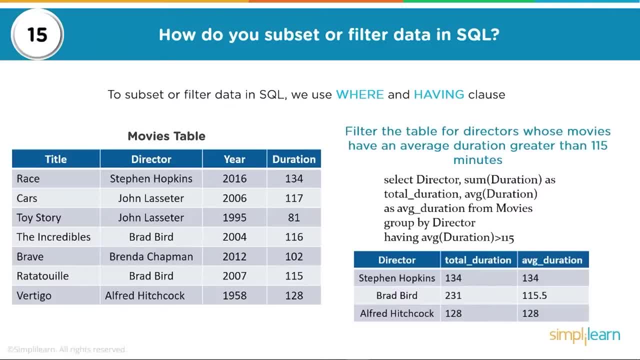 comes up and there's so many different other languages, not just my sql and not other languages, not just my sql and not other languages, not just my sql and not microsoft sql, but in addition to that microsoft sql, but in addition to that microsoft sql, but in addition to that, where the sql language comes in. 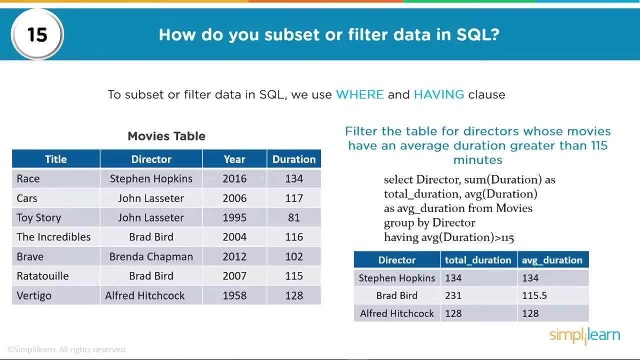 where the sql language comes in, where the sql language comes in, especially with hadoop and other areas, especially with hadoop and other areas, especially with hadoop and other areas. so you really should know your basic. so you really should know your basic. so you really should know your basic. sql doesn't hurt to get that little. 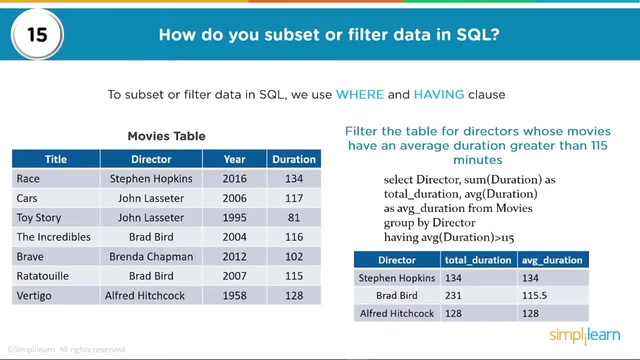 sql. doesn't hurt to get that little sql, doesn't hurt to get that little cheat sheet and glance over and double cheat sheet and glance over and double cheat sheet and glance over and double check some of the different features in check, some of the different features in. 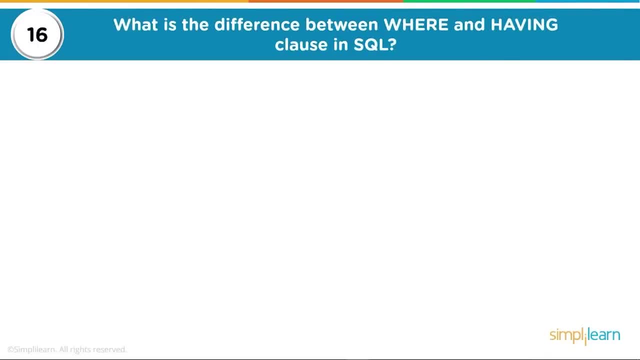 check some of the different features in sql, sql, sql. what is the difference between where and. what is the difference between where and what is the difference between where and having clause and sql. having clause and sql. having clause and sql. where, where clause works on row data in. 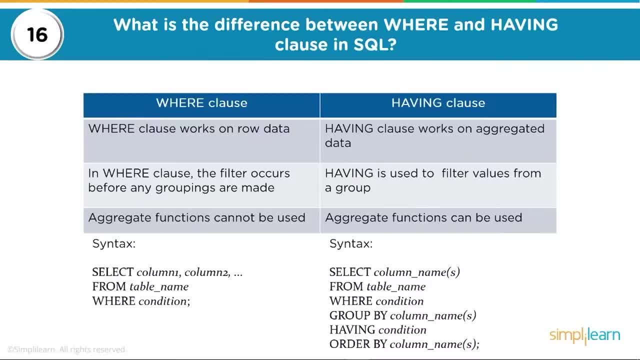 where where clause works on row data. in where where clause works on row data. in where clause the filter occurs before where clause the filter occurs before. where clause the filter occurs before. any groupings are made aggregate. any groupings are made aggregate. any groupings are made aggregate. functions cannot be used. 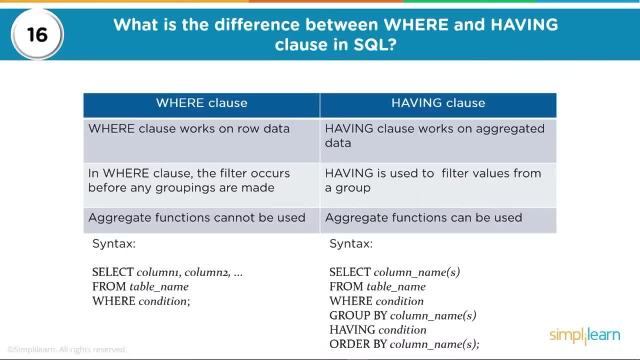 functions cannot be used. functions cannot be used, so the syntax is: select your columns. so the syntax is: select your columns. so the syntax is: select your columns from table. where what the condition is from table. where what the condition is from table. where what the condition is having clause works on aggregated data. 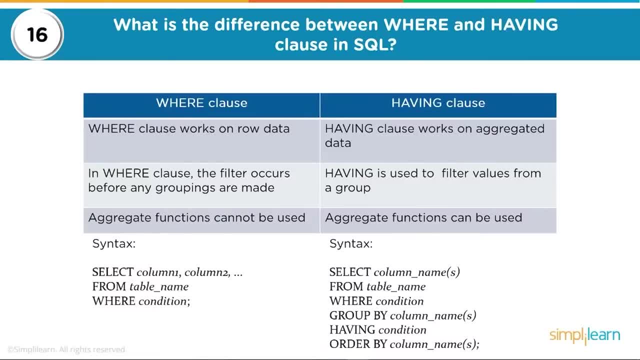 having clause works on aggregated data. having clause works on aggregated data. having is used to filter values from a having. is used to filter values from a having. is used to filter values from a group. aggregate functions can be used. group aggregate functions can be used. group aggregate functions can be used in the syntax is: select column names from: 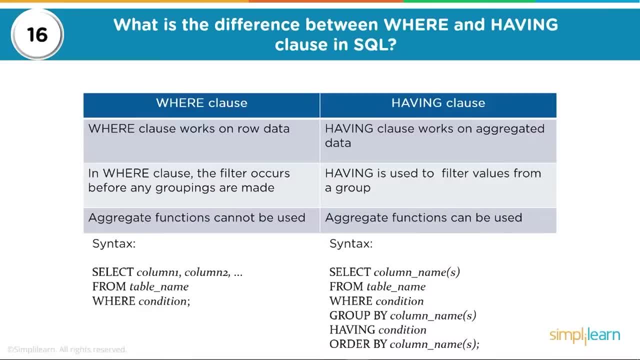 in the syntax is select column names from. in the syntax is select column names from table where the condition is. table where the condition is table where the condition is grouped by having a condition ordered by grouped. by having a condition ordered by grouped. by having a condition ordered by column names. 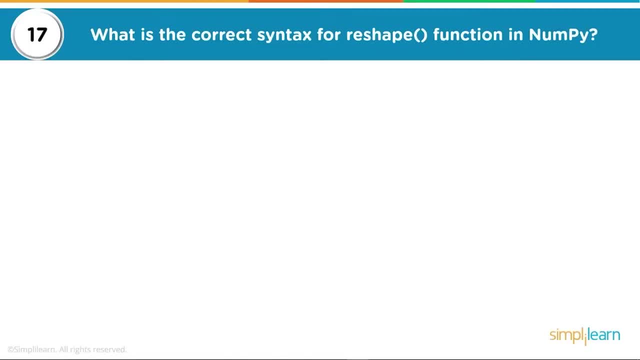 what is the correct syntax for reshape? what is the correct syntax for reshape? what is the correct syntax for reshape? function in numpy. so we're going to jump function in numpy. so we're going to jump function in numpy. so we're going to jump to the numpy array program. 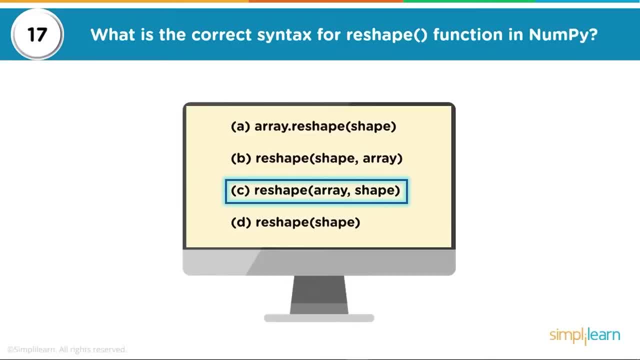 to the numpy array program, to the numpy array program, and what you come up with is you have in, and what you come up with is you have in, and what you come up with is you have, in this case it'd be numpy dot reshape a. this case it'd be numpy dot, reshape a. 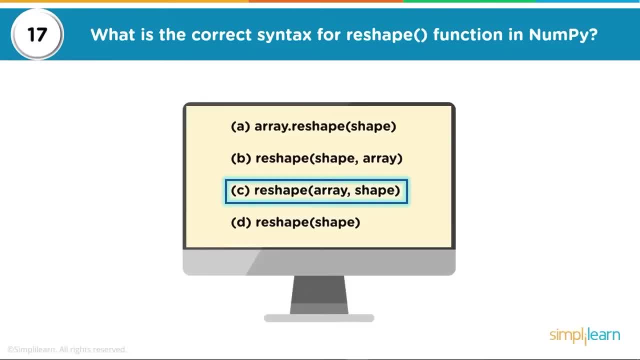 this case it'd be numpy dot reshape. a lot of times you do an import numpy. as lot of times you do an import numpy. as lot of times you do an import numpy, as in p, in p, in p- reshape and then your array and the new. reshape and then your array and the new. 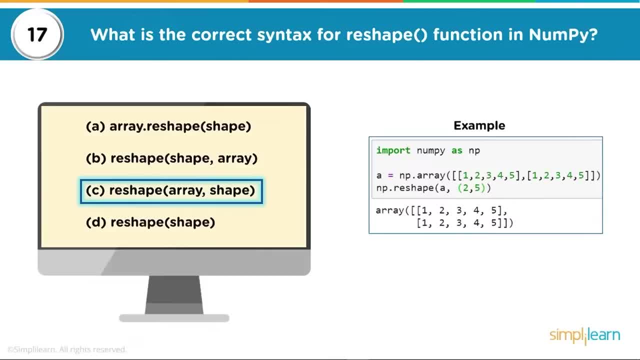 reshape, and then your array and the new shape, shape, shape. and you can see here as we as the actual, and you can see here as we as the actual and you can see here as we as the actual. example comes in: the reshape is a and. example comes in: the reshape is a and. 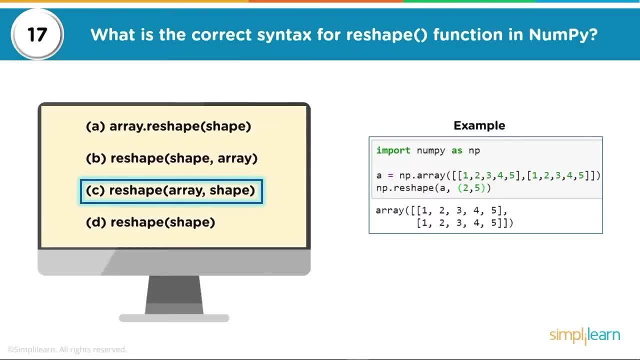 example comes in, the reshape is a and we're going to reshape it in two comma. we're going to reshape it in two comma, we're going to reshape it in two comma. five setups and you can see the printout: five setups and you can see the printout. 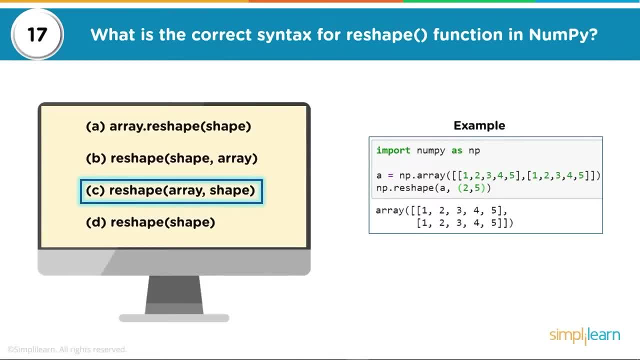 five setups and you can see the printout in there. that prints in two rows with in there, that prints in two rows with in there. that prints in two rows with five values in each one. five values in each one, five values in each one. what are the different ways to create a? 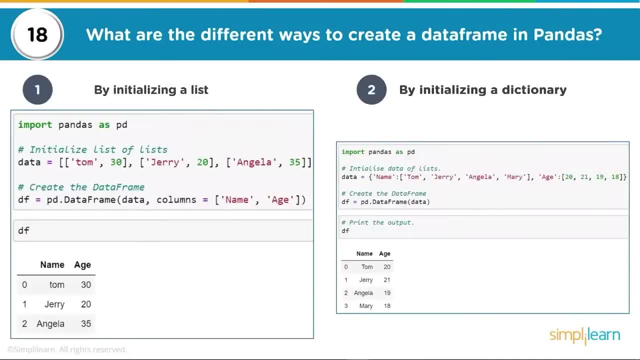 what are the different ways to create a? what are the different ways to create a data frame in pandas? data frame in pandas. data frame in pandas. well, we can do it by initializing a list. well, we can do it by initializing a list. well, we can do it by initializing a list, so you can port your pandas as pd. 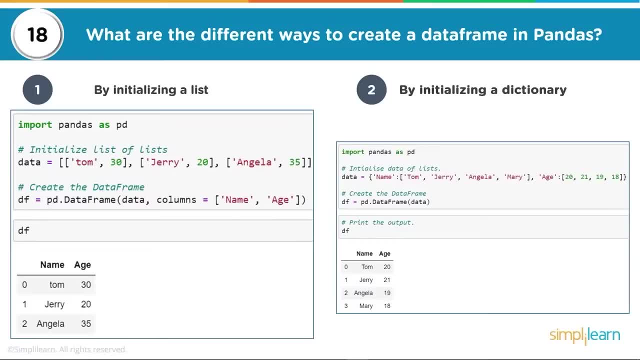 so you can port your pandas as pd. so you can port your pandas as pd. very common data equals tom 30- jerry 20. very common data equals tom 30, jerry 20. very common data equals tom 30, jerry 20, angela 35. we'll go ahead and create the. 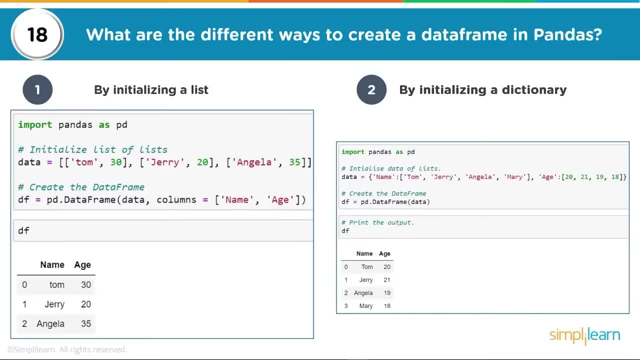 angela 35, we'll go ahead and create the angela 35. we'll go ahead and create the data frame, data frame, data frame and we'll say pddataframe is the data and we'll say pddataframe is the data and we'll say pddataframe is the data. columns equals name and age, so you can. 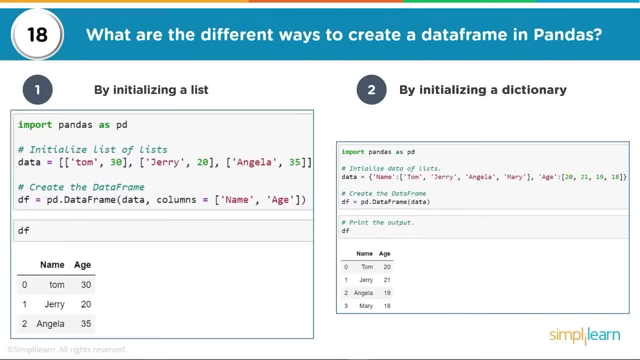 columns equals name and age, so you can. columns equals name and age, so you can designate your columns. you can also. it designate your columns, you can also it designate your columns, you can also. it is a index in there, you should always. is a index in there, you should always. 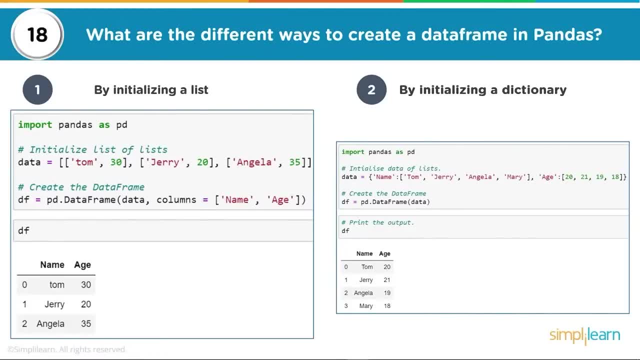 is a index in there. you should always remember that the index. remember that the index. remember that the index in this case. maybe you want the index in this case. maybe you want the index in this case. maybe you want the index instead of one, two to be, instead of one, two to be. 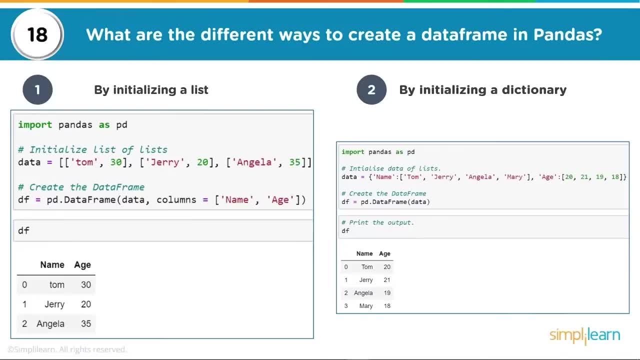 instead of one, two to be the date they signed up, or who knows you the date they signed up, or who knows you the date they signed up, or who knows you know whatever and you can see right know whatever, and you can see right, know whatever and you can see right there, it just generates a nice pandas. 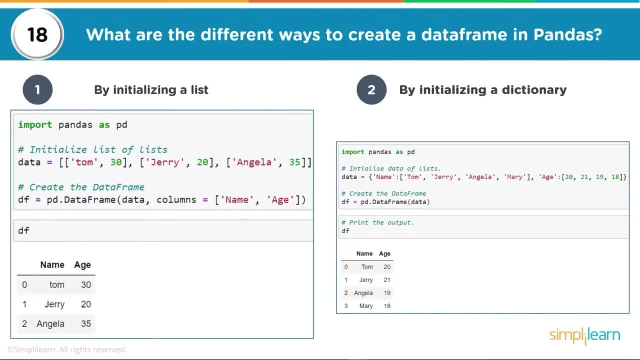 Name and age So you can designate your columns. You can also. it is an index in there. You should always remember that the index- in this case maybe you want the index instead of 1,, 2, to be the date they signed up, or who knows, you know whatever. 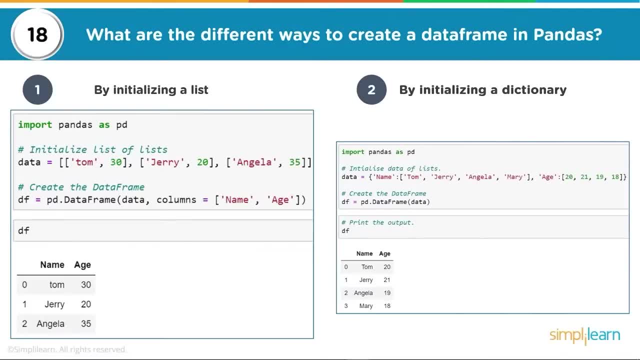 And you can see right there it just generates a nice Pandas data frame with Tom, Jerry and Angela. Another way you can initialize a data frame is from dictionary. You can see here we have a dictionary where the date equals name: Tom Jerry, Angela, Mary. 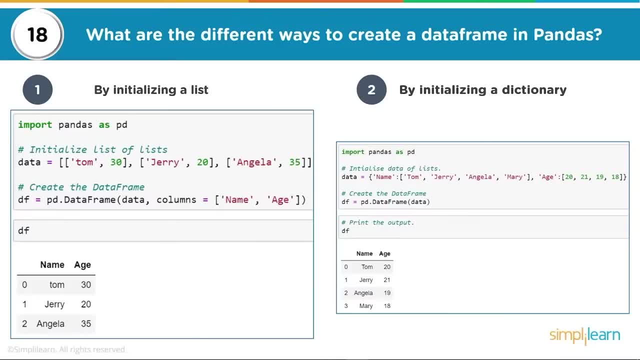 Age is 20,, 21,, 19,, 18, and if we do a dfpddataFrame on the data, you'll get a nice, the same kind of setup. You get your name, age, Tom, Jerry, Angela and Mary. 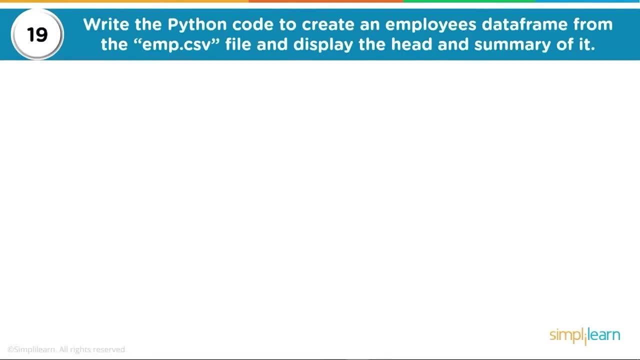 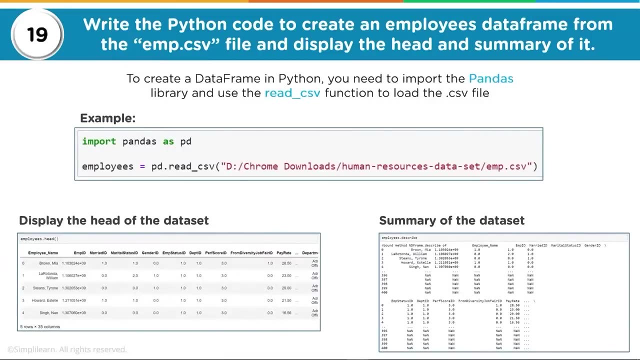 Write the Python code to create an employee's data frame from the empcsv file and display the head and summary of it. To create a data frame in Python, you need to import the Pandas library and use the read CSV function to load the CSV file. 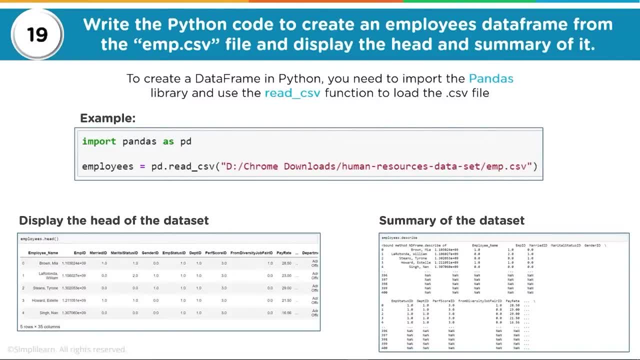 And here you can see we have import Pandas as pd employees, or the data frame employees equals pdreadcsv. and then you have your path to that CSV file. There's a number of settings in the read CSV where you can tell it how many rows are the top index. 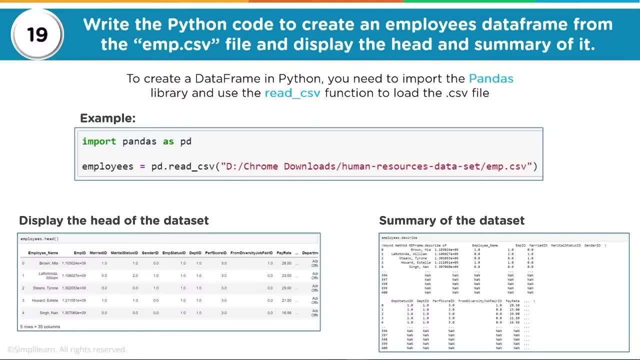 You can set the columns in there. You can have skip rows, There's all kinds of things. you can also go in there and double check with your read CSV, But the most basic one is just to read a basic CSV. How will you select the department and age columns from an employee's data frame? 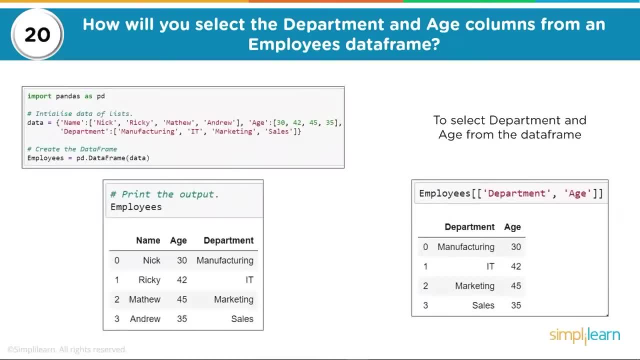 So we have import Pandas as pd. You can see we have created our data. We will go ahead and create our employee's pd data frame on the left And then on the right to select department and age from the data frame. we just do employees. 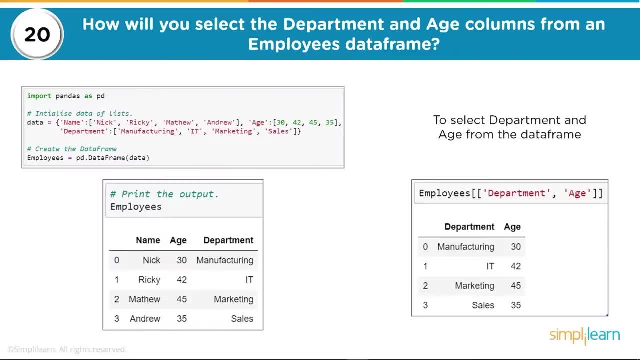 You put the brackets around it. Now, if you're just doing one column you could do just department. But if you're doing multiple columns you've got to have those in a second set of brackets. It's got to be a reference with a list within the reference. 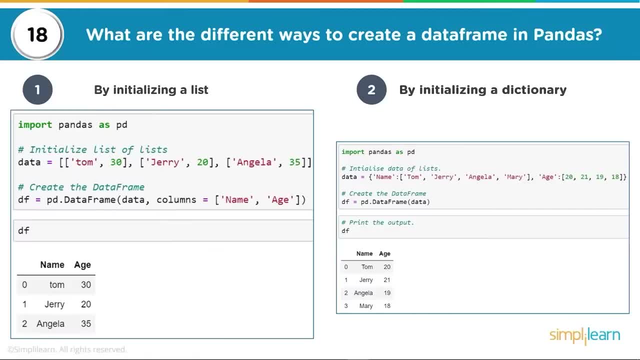 there it just generates a nice pandas there it just generates a nice pandas data frame with tom data frame with tom data frame with tom, jerry and angela. another way you can jerry and angela. another way you can jerry and angela. another way you can initialize a. 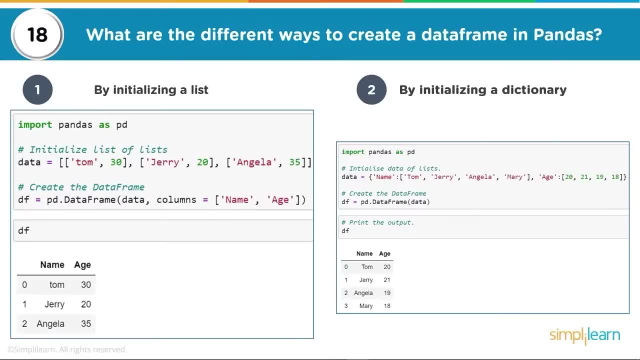 initialize a. initialize a data frame is from dictionary. you can see data frame is from dictionary. you can see data frame is from dictionary. you can see, here we have a dictionary. here we have a dictionary. here we have a dictionary where the date equals name: tom jerry. 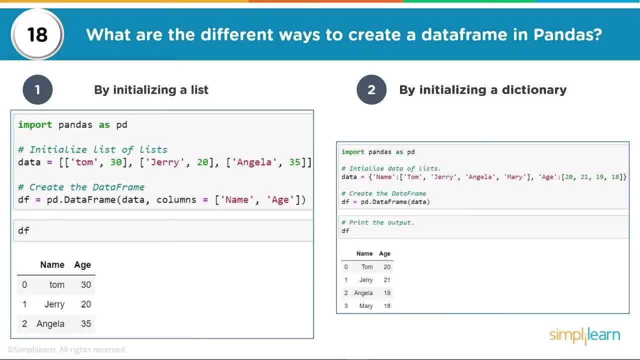 where the date equals name tom jerry. where the date equals name tom jerry. angela mary age is 2021- 1918. and if we angela mary age is 2021- 1918. and if we angela mary age is 2021- 1918. and if we do a dfpd. 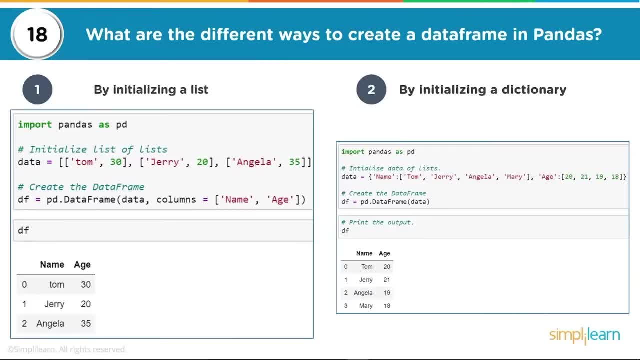 do a dfpd, do a dfpd data frame on the data. you'll get a nice data frame on the data. you'll get a nice data frame on the data. you'll get a nice the same kind of setup. you get your name. the same kind of setup. you get your name. 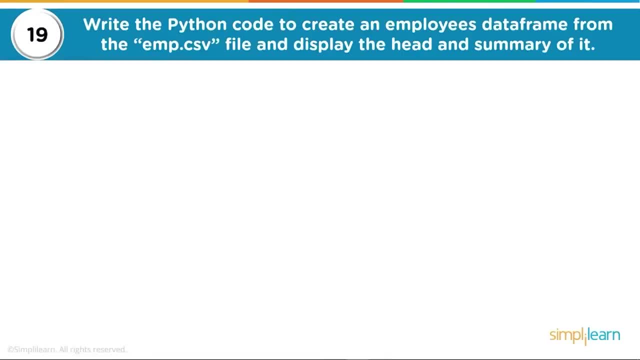 the same kind of setup. you get your name: age tom, jerry, angela and mary. age tom, jerry, angela and mary. age tom, jerry, angela and mary. write the python code to create an. write the python code to create an. write the python code to create an employee's data frame from the empcsv. 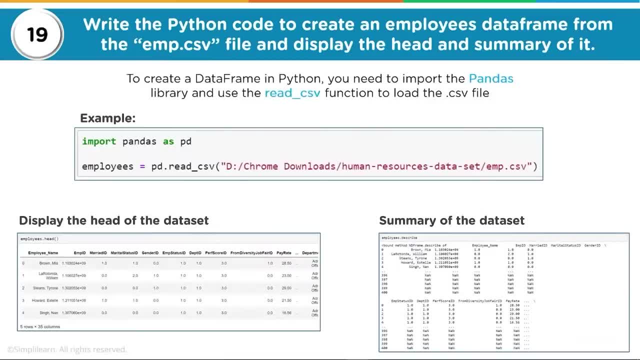 employee's data frame from the empcsv, employee's data frame from the empcsv file and display the head and summary of file. and display the head and summary of file and display the head and summary of it. it it to create a data frame in python. you. 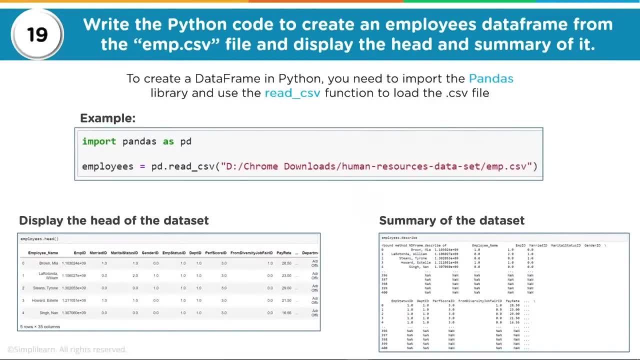 to create a data frame in python. you to create a data frame in python. you need to import the pandas library and need to import the pandas library. and need to import the pandas library and use the read csv function to load the csv. use the read csv function to load the csv. 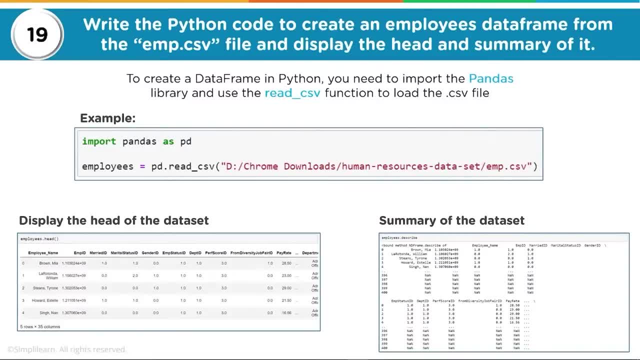 use the read csv function to load the csv file, file, file. and here you can see we have import. and here you can see we have import. and here you can see we have import: pandas as pd employees, pandas as pd employees, pandas as pd employees, or the data frame employees equals pd. 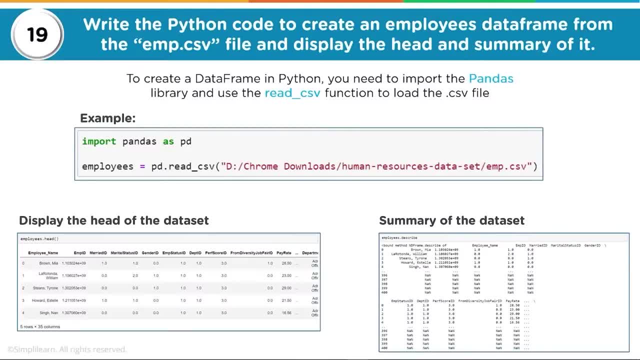 or the data frame employees equals pd. or the data frame employees equals pd. dot read csv. dot read csv. dot read csv. and then you have your path to that csv and then you have your path to that csv and then you have your path to that csv file. 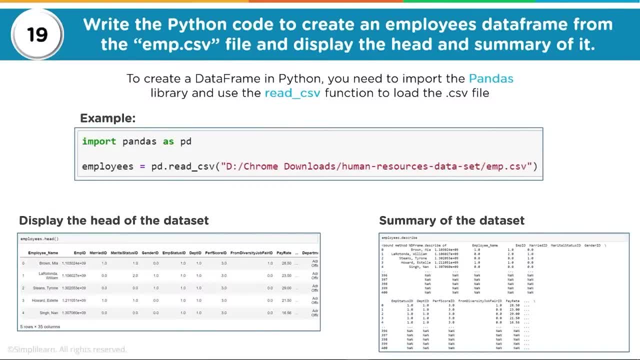 file, file. there's a number of settings in the read. there's a number of settings in the read. there's a number of settings in the read: csv, where you can tell it how many csv. where you can tell it how many csv. where you can tell it how many rows are the top index. 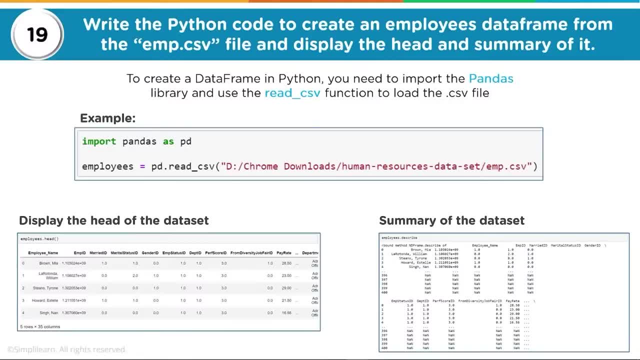 rows are the top index. rows are the top index. you can set the columns in there. you can set the columns in there. you can set the columns in there. you can have skip rows. there's all kinds. you can have skip rows. there's all kinds. you can have skip rows. there's all kinds of things. you can also go in there and 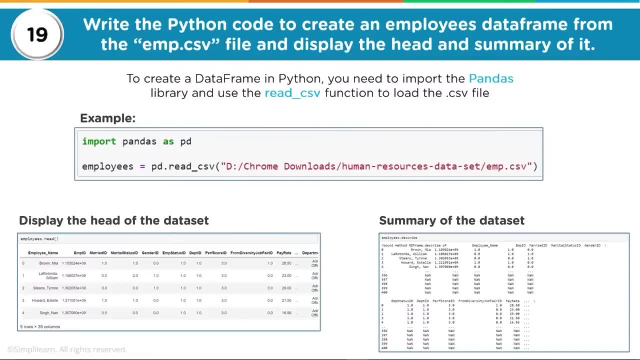 of things you can also go in there, and of things you can also go in there and double check with your read csv. but the double check with your read csv, but the double check with your read csv, but the most basic one is just to read a basic. 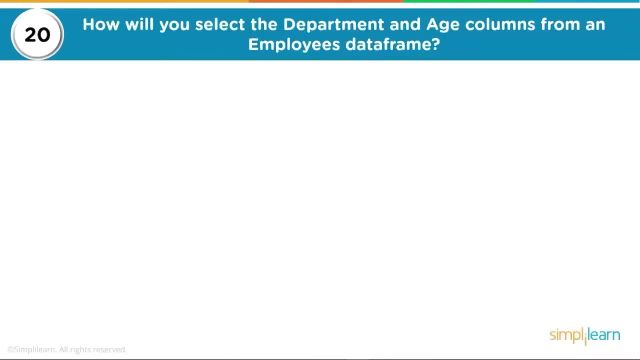 most basic one is just to read a basic. most basic one is just to read a basic: csv, csv, csv. how will you select the department and how will you select the department and how will you select the department and age columns from an employee's data. age columns from an employee's data. 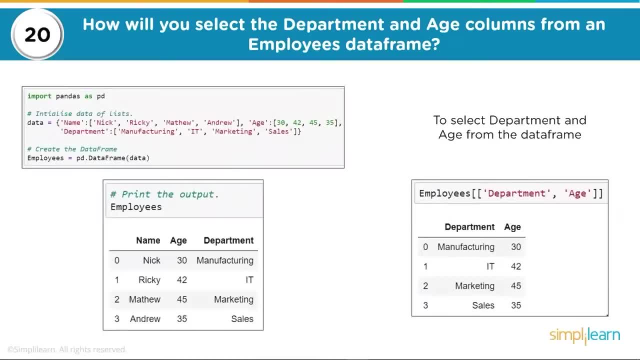 age columns from an employee's data frame frame frame. so we have import pandas as pd. you can. so we have import pandas as pd, you can. so we have import pandas as pd. you can see, we have created our data. see, we have created our data. see, we have created our data. we will go ahead and create our. 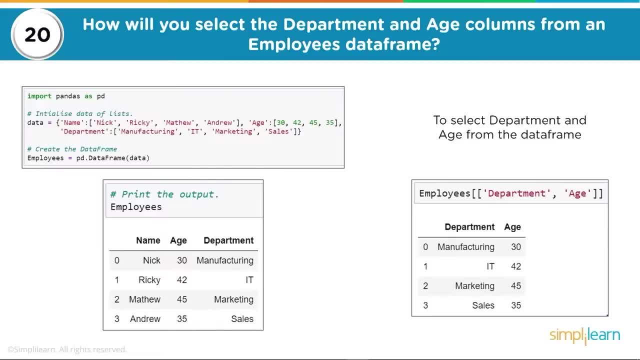 we will go ahead and create our. we will go ahead and create our employees pd data frame on the left. employees pd data frame on the left. employees pd data frame on the left, and then on the right to select, and then on the right to select, and then on the right to select department and aids from the data frame. 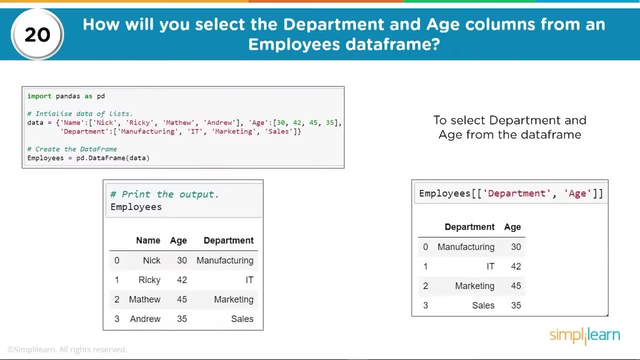 department and aids from the data frame department and aids from the data frame. we just do employees and you put the we just do employees and you put the we just do employees. and you put the brackets around it. now, if you're just brackets around it, now, if you're just. 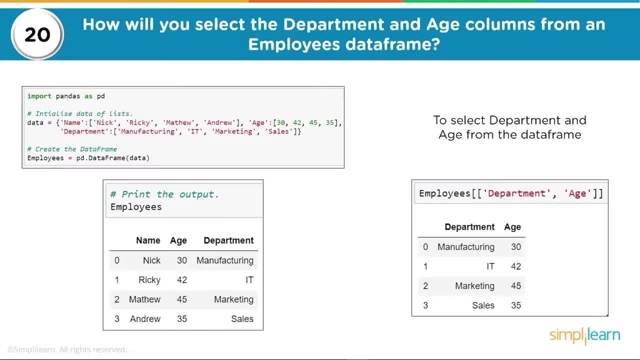 brackets around it. now, if you're just doing one column, you could do just doing one column. you could do just doing one column. you could do just department. but if you're doing multiple department, but if you're doing multiple department, but if you're doing multiple columns, you got to have those in a. 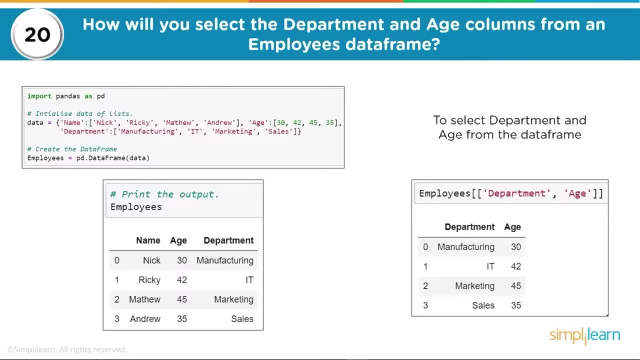 columns. you got to have those in a columns. you got to have those in a second set of brackets. it's got to be a second set of brackets. it's got to be a second set of brackets. it's got to be a reference with a list within the 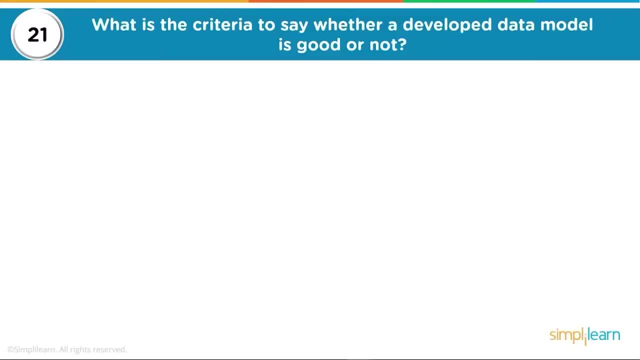 reference, with a list within the reference, with a list within the reference, reference reference. what is the criteria to say whether a? what is the criteria to say whether a? what is the criteria to say whether a developed data model is good or not? developed data model is good or not. 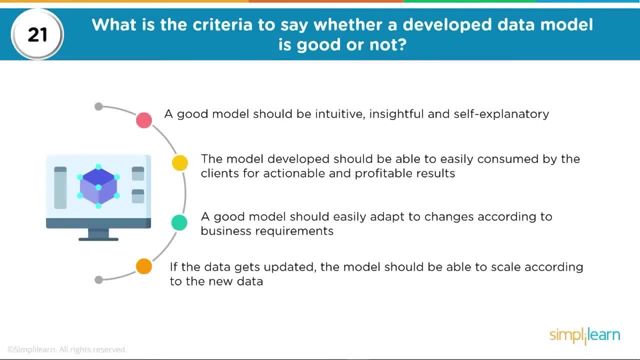 developed data model is good or not. a good model should be intuitive. a good model should be intuitive. a good model should be intuitive, insightful and self-explanatory. insightful and self-explanatory, insightful and self-explanatory. follow the old saying: kiss, keep it. follow the old saying: kiss, keep it. 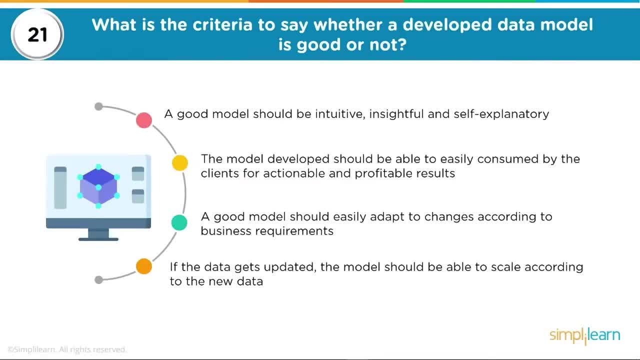 follow the old saying: kiss. keep it simple, simple, simple. the model developed should be able to. the model developed should be able to. the model developed should be able to easily consumed by the clients. for easily consumed by the clients, for easily consumed by the clients, for actionable and profitable results. 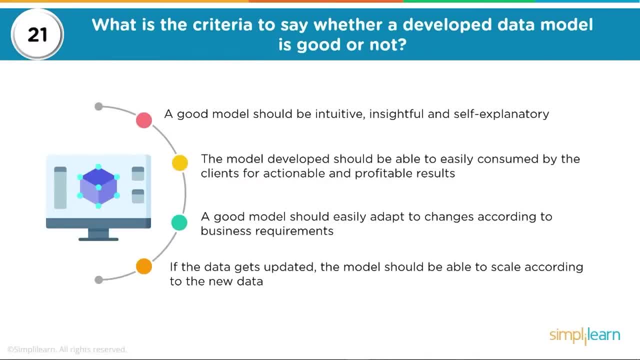 actionable and profitable results. actionable and profitable results. so if they can't read it, what good is so if they can't read it? what good is so if they can't read it? what good is it? a good model should easily adapt to it. a good model should easily adapt to. 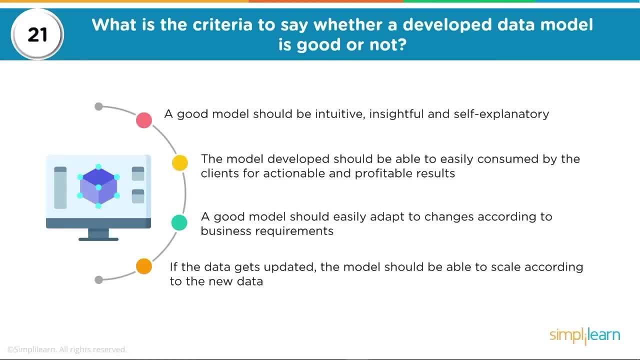 it. a good model should easily adapt to changes according to business changes, according to business changes, according to business requirements, requirements, requirements. we live in quite a dynamic world. we live in quite a dynamic world. we live in quite a dynamic world nowadays, so that's pretty self-evident. 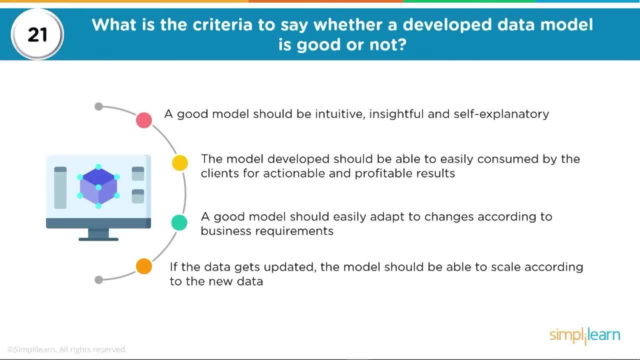 nowadays. so that's pretty self-evident nowadays. so that's pretty self-evident and if the data gets updated, the model and if the data gets updated, the model and if the data gets updated, the model should be able to scale accordingly to, should be able to scale accordingly to. 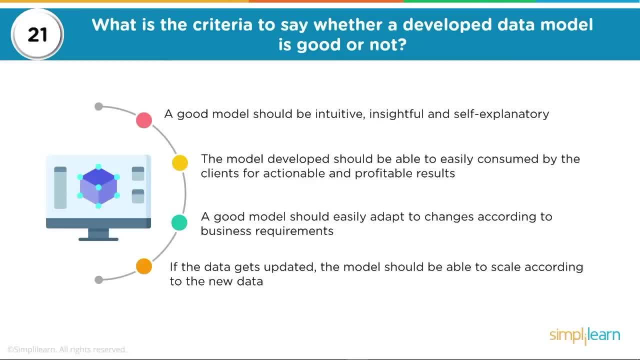 should be able to scale accordingly to the new data. so you have a nice data, the new data, so you have a nice data. the new data, so you have a nice data. pipeline going where when something. when pipeline going where when something. when pipeline going where when something. when you get new data coming in, you don't 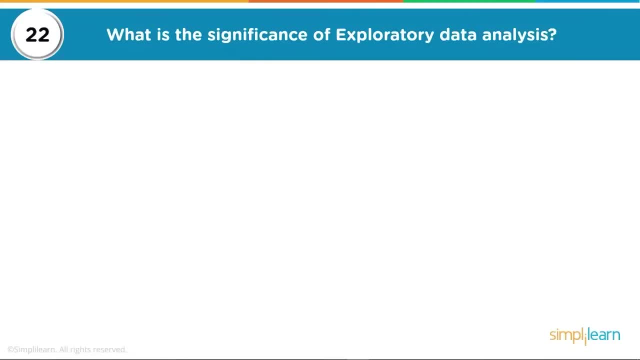 you get new data coming in? you don't. you get new data coming in. you don't have to go and rewrite the whole code. have to go and rewrite the whole code. have to go and rewrite the whole code. what is the significance of exploratory? what is the significance of exploratory? 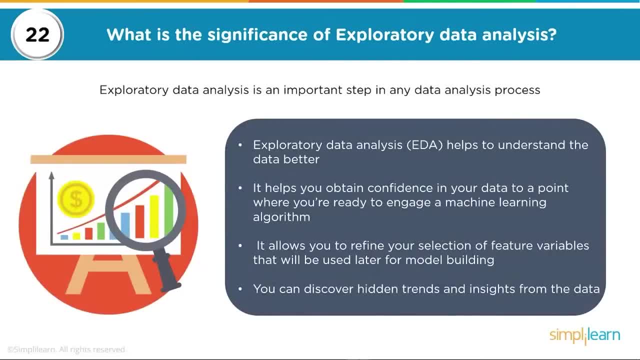 what is the significance of exploratory data analysis, data analysis, data analysis, exploratory data analysis is an exploratory data analysis, is an exploratory data analysis. is an important step in any data analysis, important step in any data analysis, important step in any data analysis process process. 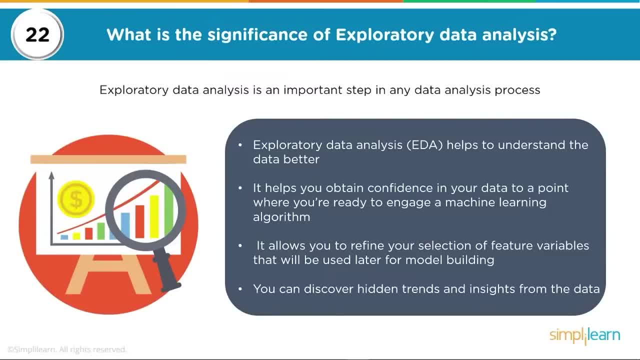 process. exploratory data analysis. eda helps to exploratory data analysis. eda helps to exploratory data analysis. eda helps to understand the data better. it helps you understand the data better. it helps you understand the data better. it helps you obtain confidence in your data to a point. 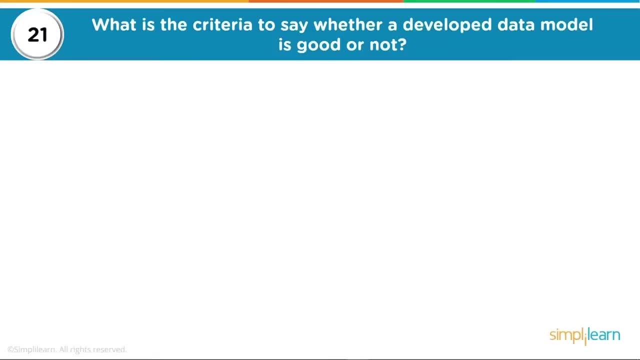 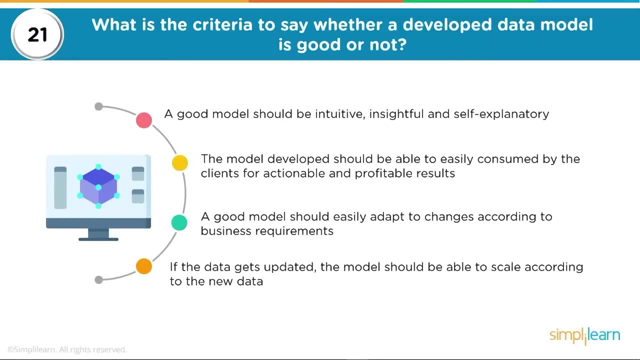 What is the criteria to say whether a developed data model is good or not? A good model should be intuitive, insightful and self-explanatory. Follow the old saying KISS, keep it simple. The model developed should be able to easily be consumed by the clients for actionable and profitable results. 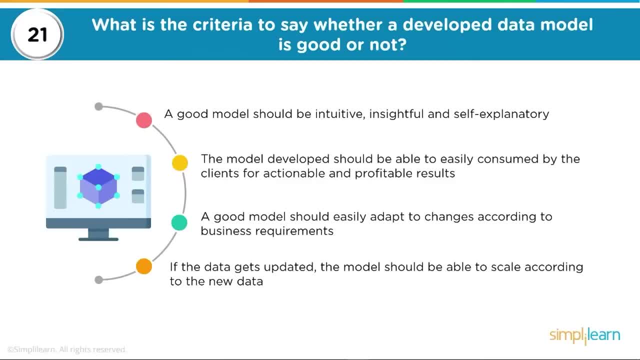 So if they can't read it, what good is it? A good model should easily adapt to changes according to business requirements. We live in quite a dynamic world nowadays, so it's pretty self-evident. And if the data gets updated, the model should be able to scale accordingly to the new data. 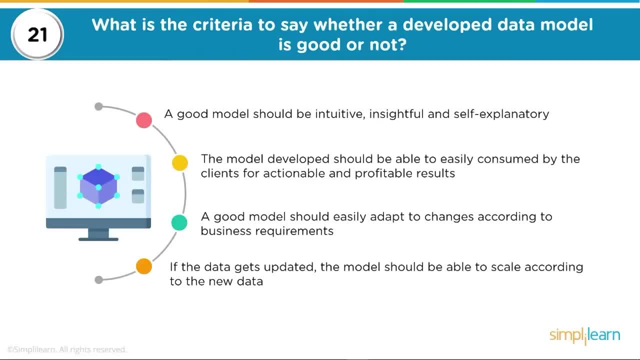 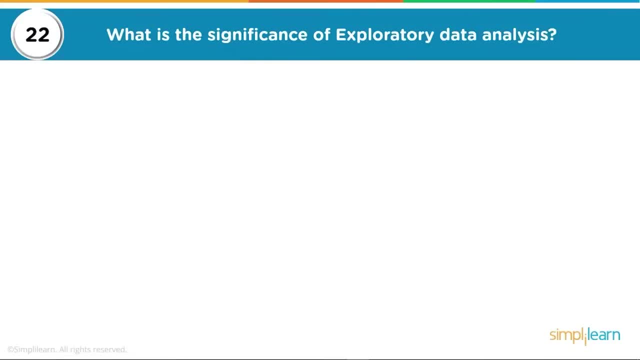 So you have a nice data pipeline going where, when something, when you get new data coming in, you don't have to go and rewrite the whole code. What is the significance of exploratory data analysis? Exploratory data analysis is an important step. 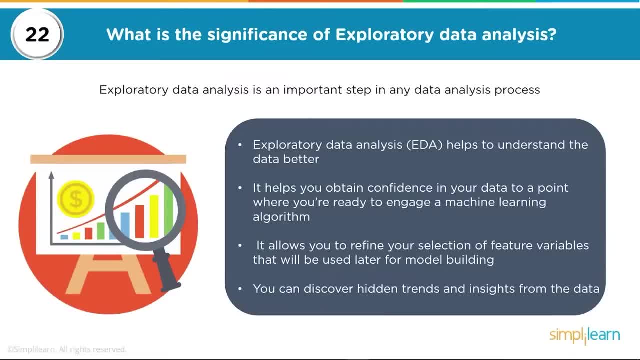 Exploratory data analysis is an important step in any data analysis process. Exploratory data analysis- EDA- helps to understand the data better. It helps you obtain confidence in your data to a point where you're ready to engage a machine learning algorithm. 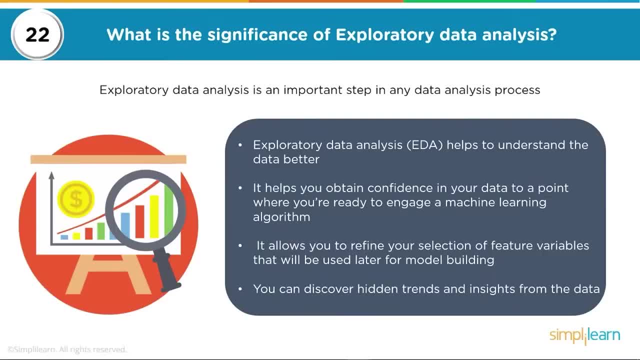 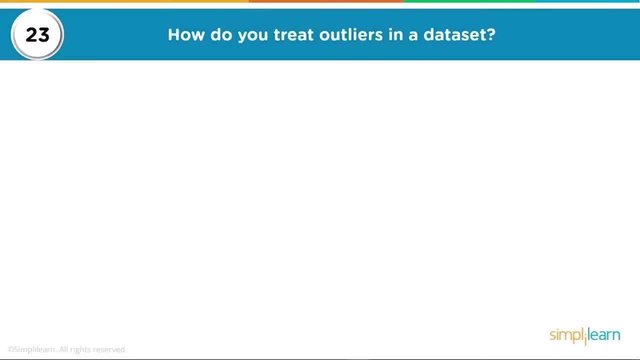 It allows you to refine your selection of feature variables that will be used later for model building. You can discover hidden trends and insights from the data. How do you treat outliers in a data set? An outlier is a data point that is distant from other similar points. 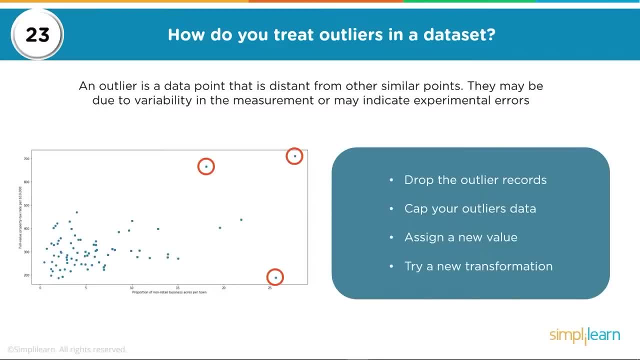 An outlier is a data point that is distant from other similar points. They may be due to variability in the measurement or may indicate experimental errors. One: you can drop the outlier records. Pretty straightforward. You can cap your outlier's data so it doesn't go past a certain value. 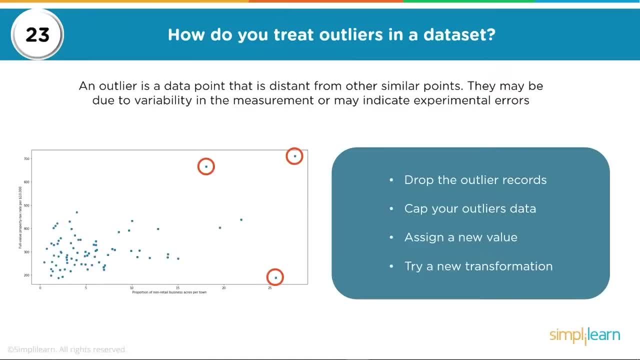 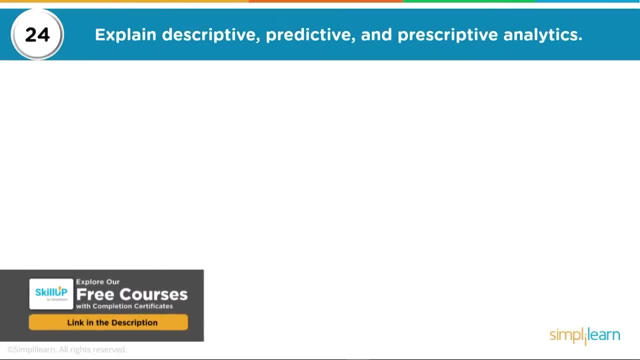 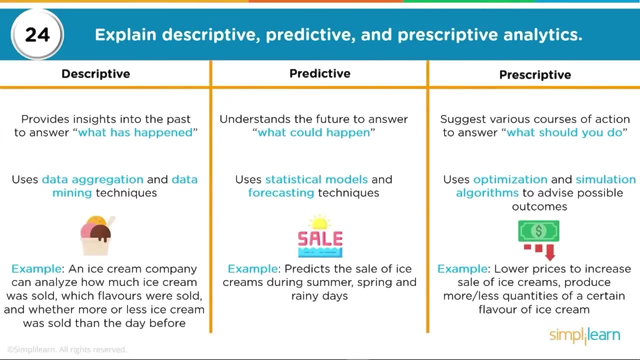 You can assign it a new value. You can also try a new transformation to see if those outliers come in if you transform it slightly differently. Explain descriptive, predictive and prescriptive analytics. Descriptive provides insights into the past to answer what has happened. 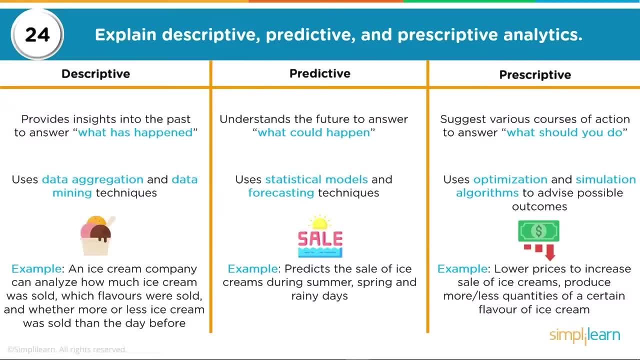 Uses data aggregation and data mining techniques. Examples: an ice cream company can analyze how much ice cream was sold, which flavors were sold and whether more or less ice cream was sold than before. Predictive: understands the future to the answer: What could happen? 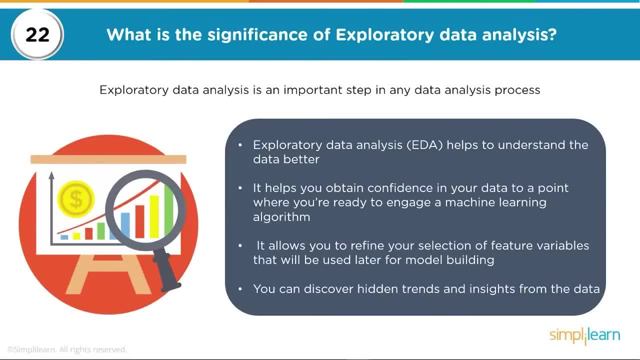 obtain confidence in your data to a point. obtain confidence in your data to a point where you're ready to engage. where you're ready to engage, where you're ready to engage- a machine learning algorithm. it allows a machine learning algorithm. it allows a machine learning algorithm. it allows you to refine your selection of feature. 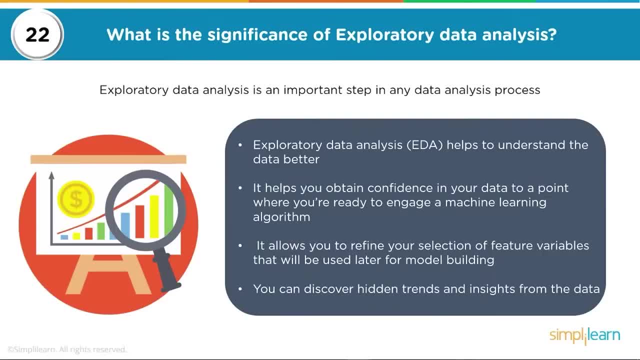 you to refine your selection of feature. you to refine your selection of feature variables that will be used later, for variables that will be used later, for variables that will be used later for model building, model building, model building: you can discover hidden trends. and you can discover hidden trends and. 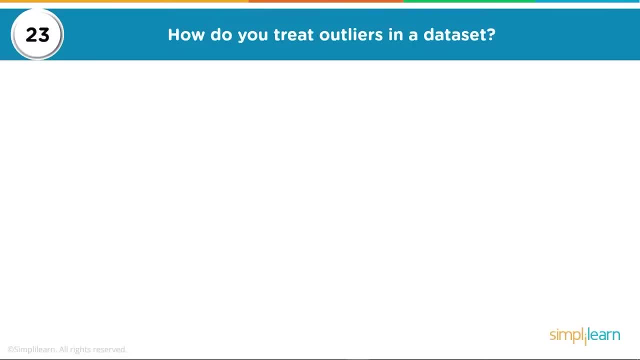 you can discover hidden trends and insights from the data. insights from the data. insights from the data. how do you treat outliers in a data? how do you treat outliers in a data? how do you treat outliers in a data set set set? an outlier is a data point that is. 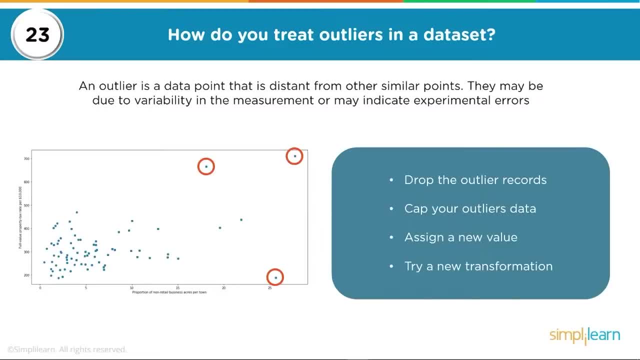 an outlier is a data point that is an outlier is a data point that is distant from other similar points. they distant from other similar points. they distant from other similar points. they may be due to variability in the, may be due to variability in the, may be due to variability in the measurement, or may indicate experimental. 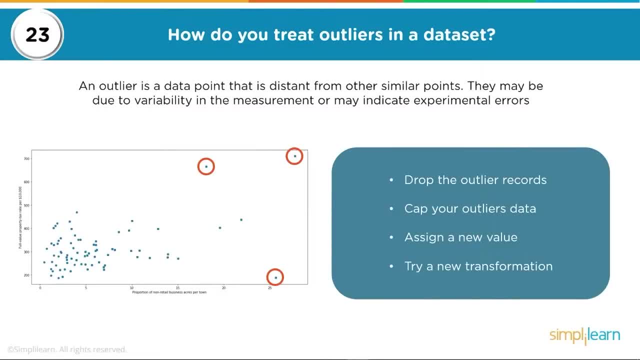 measurement, or may indicate experimental measurement, or may indicate experimental errors, errors, errors. one: you can drop the outlier records. one: you can drop the outlier records. one: you can drop the outlier records pretty straightforward. you can cap your pretty straightforward. you can cap your pretty straightforward. you can cap your outliers data. 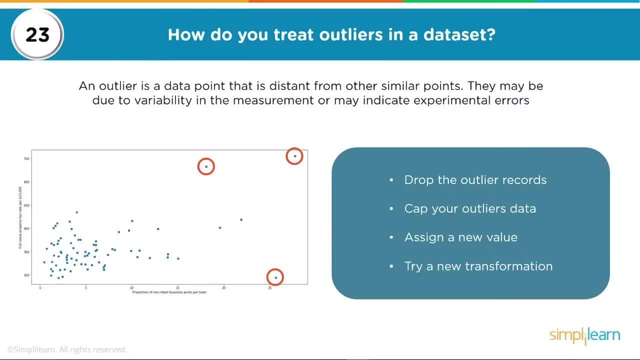 outliers data. outliers data, so it doesn't go past a certain value. so it doesn't go past a certain value. so it doesn't go past a certain value. you can assign it a new value. you can assign it a new value. you can assign it a new value. you can also try a new transformation to. 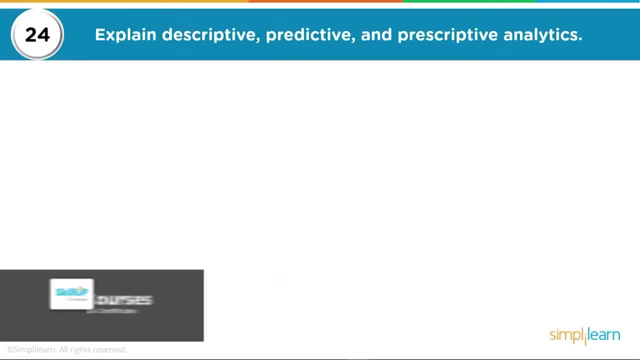 you can also try a new transformation to. you can also try a new transformation to see if those outliers come in. if you see if those outliers come in. if you see if those outliers come in, if you transform it slightly differently, transform it slightly differently, transform it slightly differently, explain descriptive, predictive and 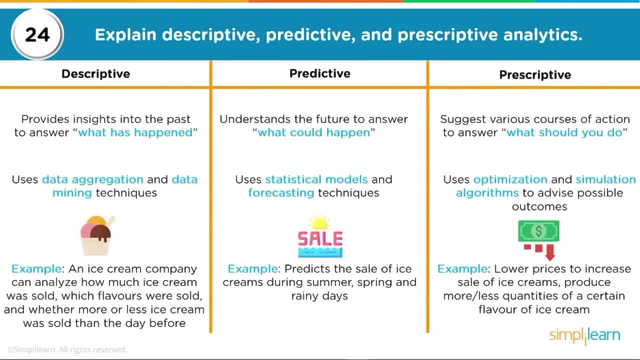 explain descriptive, predictive. and explain descriptive, predictive and prescriptive analytics. prescriptive analytics: prescriptive analytics: descriptive provides insights into the descriptive. provides insights into the descriptive. provides insights into the past to answer what has happened past. to answer what has happened past. to answer what has happened. uses data aggregation and data mining. 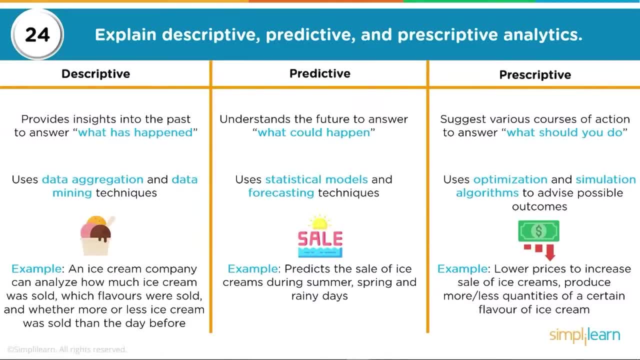 uses data aggregation and data mining. uses data aggregation and data mining techniques. examples: an ice cream company techniques. examples: an ice cream company techniques. examples: an ice cream company can analyze how much ice cream was sold. can analyze how much ice cream was sold. can analyze how much ice cream was sold, which flavors were sold. 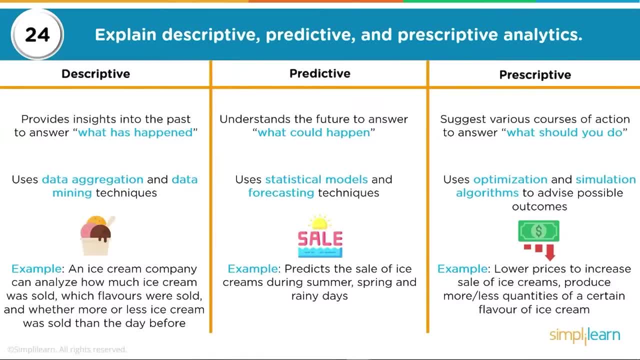 which flavors were sold, which flavors were sold and whether more or less ice cream was, and whether more or less ice cream was, and whether more or less ice cream was sold than before sold than before. sold than before. predictive understands the future to the. predictive. understands the future to the. 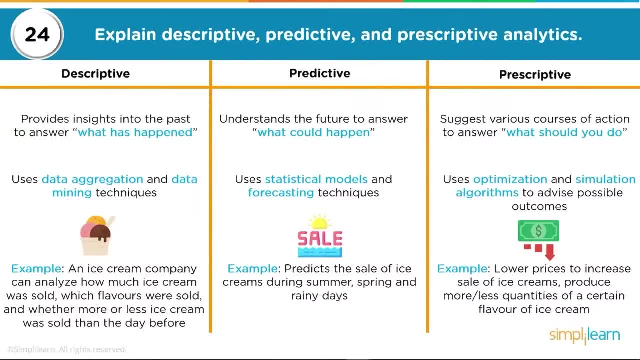 predictive: understands the future. to the answer what could happen uses statistical answer: what could happen: uses statistical answer: what could happen: uses statistical models and forecasting techniques. models and forecasting techniques. models and forecasting techniques. example: predicts the sale of ice creams. example: predicts the sale of ice creams. example: predicts the sale of ice creams during the summer, spring and rainy days. 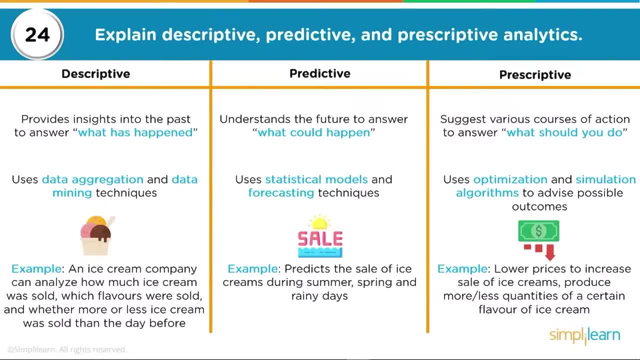 during the summer, spring and rainy days during the summer, spring and rainy days. so this is always interesting because you so this is always interesting because you so this is always interesting because you have your descriptive which comes in, and have your descriptive which comes in, and have your descriptive which comes in and your businesses are always looking to. 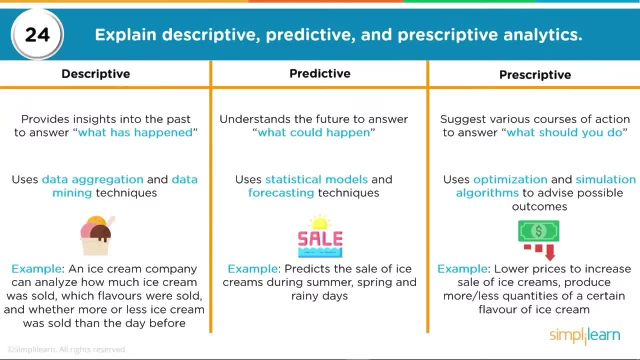 Uses statistical models and forecasting techniques. Example: predicts the sale of ice creams during the summer, Spring and rainy days. So this is always interesting because you have your descriptive which comes in and your businesses are always looking to know what happened. Hey, did we have good sales last quarter? 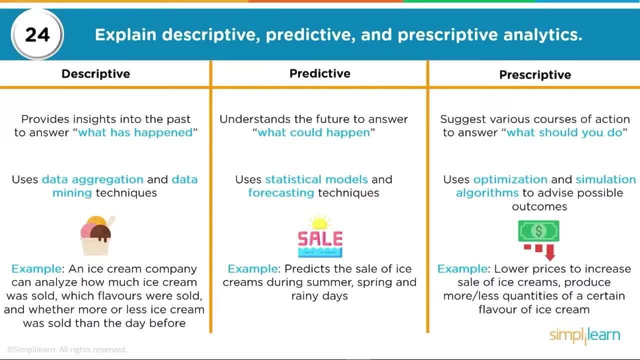 What are we expecting next quarter in the sales? And we have a huge jump when we do prescriptive. Suggest various courses of action to answer: what should you do? Uses optimization and simulation algorithms to advise possible outcomes. Example: lower prices to increase sales. 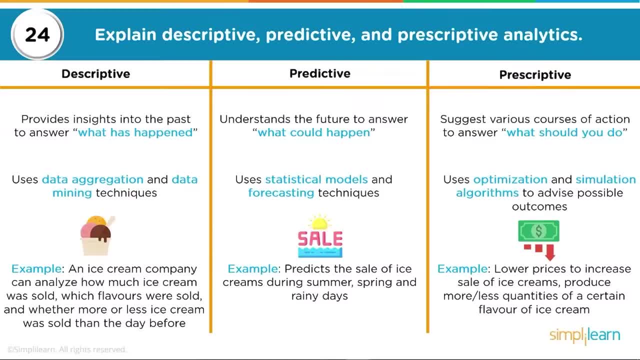 Unstable prices to increase sales, Correct price to be lost in the market. Now you could use a descriptive on your best example Example: how many people have been infected, What's happened. And you could see the same in your previous example. 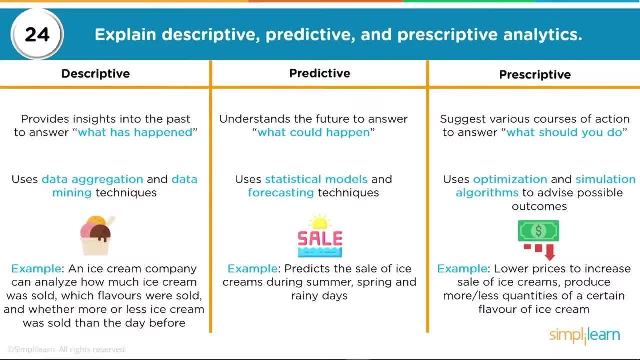 How many people have been affected And how many people have died in an area. What does the prescriptive look like? Next prescriptive: What can we change in our distinguishing model of how to do a better job? What can we change in our setup to have a better outcome? 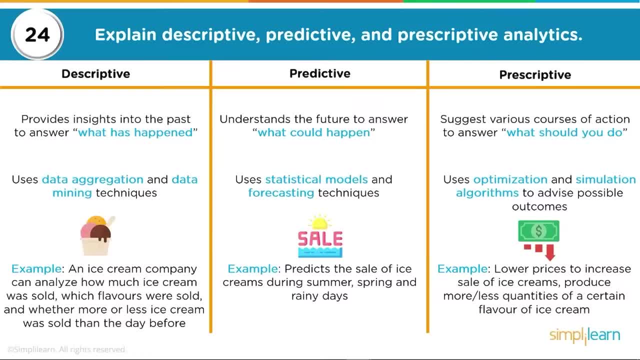 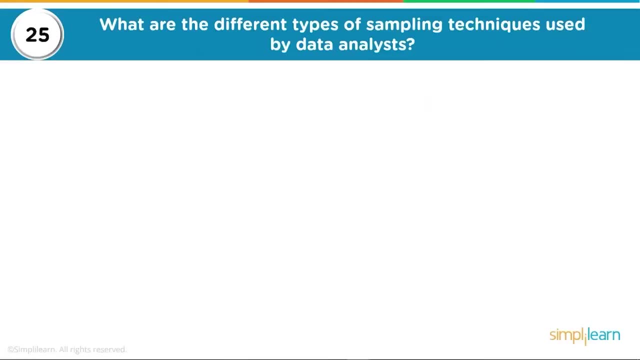 Maybe if we did more social distancing, if we tracked the virus. How do these different things directly affect the end and can we create a better ending by changing some underlying criteria? What are the different types of sampling techniques used by data analysis? Sampling is a statistical method to select a subset of data from an entire data set. 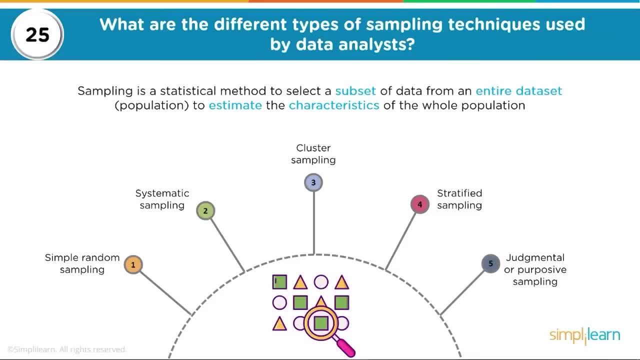 Population. to estimate the characteristics of the whole population One, we can do a simple random sampling. so we can just pick out 500 random people in the United States to sample them. They call it a population in regular data. We also call that a population just because that's where it came from- was mainly from doing census. 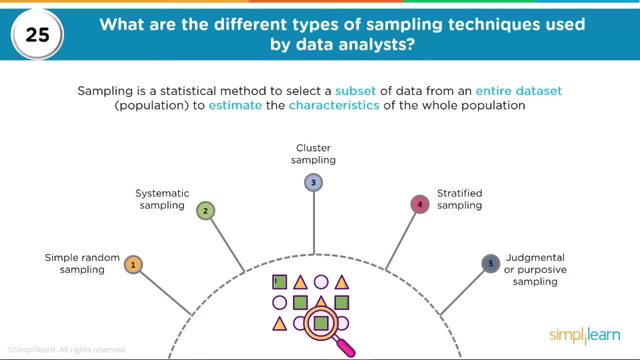 systematic sampling, cluster sampling, stratified sampling and judgment or purposive sampling. Then we have our systematic sampling. That's where you're doing like using 1, 5, 10, 15, 20. use a very systematic approach for pulling samples from the setup: cluster sampling. 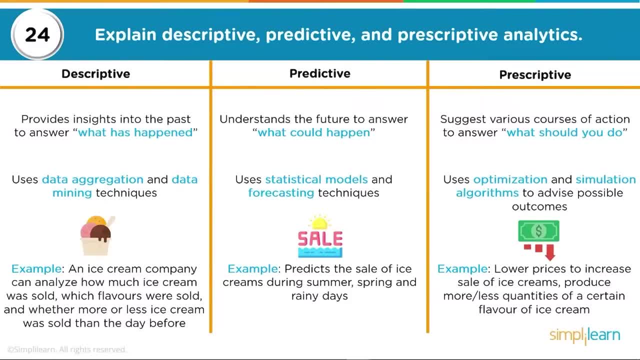 your businesses are always looking to. your businesses are always looking to know what happened. hey, did we have good know what happened? hey, did we have good know what happened? hey, did we have good cells last quarter? what are we expecting cells last quarter? what are we expecting cells last quarter? what are we expecting next quarter in the cells? and we have a 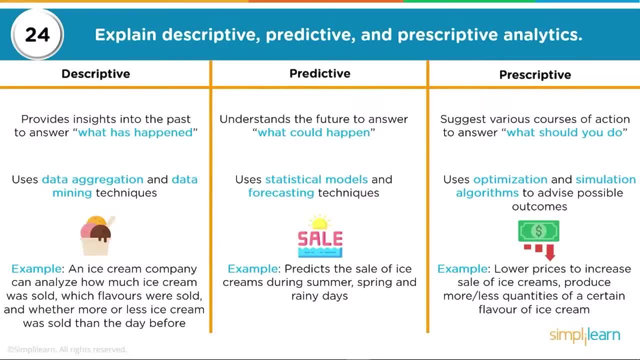 next quarter in the cells and we have a next quarter in the cells and we have a huge jump when we do prescriptive, huge jump when we do prescriptive, huge jump when we do prescriptive. suggest various courses of action. to suggest various courses of action to. 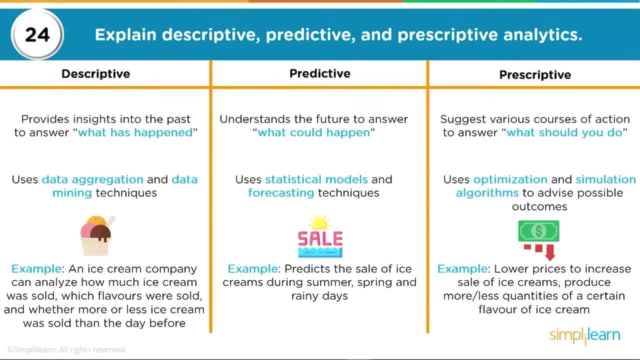 suggest various courses of action. to answer: what should you do? uses answer: what should you do? uses answer: what should you do? uses optimization and simulation algorithms: to optimization and simulation algorithms. to optimization and simulation algorithms to advise possible outcomes example: lower. advise possible outcomes example: lower. advise possible outcomes example: lower prices to increase. 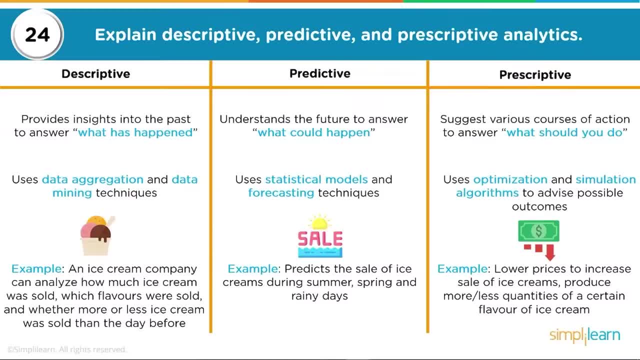 prices. to increase prices to increase cell of ice creams produce more or less. cell of ice creams produce more or less. cell of ice creams produce more or less quantities of certain flavor of ice, quantities of certain flavor of ice, quantities of certain flavor of ice cream. and we can certainly uh today's. 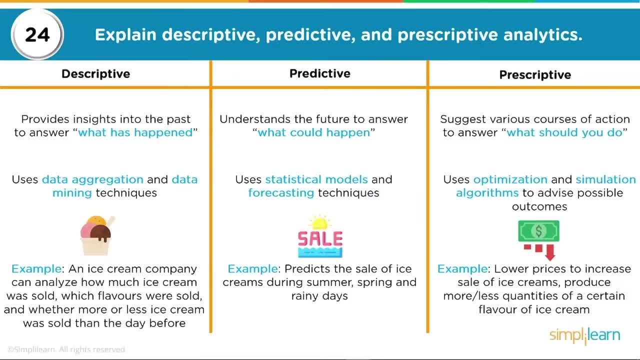 cream and we can certainly uh today's cream and we can certainly uh today's world with the covet virus, because we world with the covet virus, because we world with the covet virus, because we had that in our earlier graph. you could. had that in our earlier graph, you could. 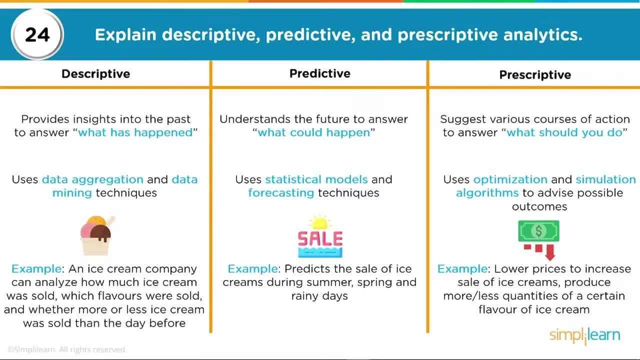 had that in our earlier graph. you could see that as a descriptive. what's see that as a descriptive? what's see that as a descriptive? what's happened? how many people have been happened? how many people have been happened? how many people have been infected? how many people have died in an 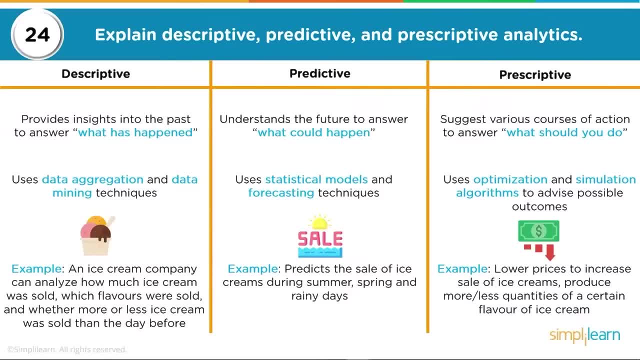 infected. how many people have died in an infected? how many people have died in an area, area, area, predictive? where do we predict that to go? predictive? where do we predict that to go? predictive? where do we predict that to go? do we see it's going to get worse, is it? do we see it's going to get worse? is it? do we see it's going to get worse? is it going to get better? what do we predict going to get better? what do we predict going to get better? what do we predict that we're going to need in hospital? 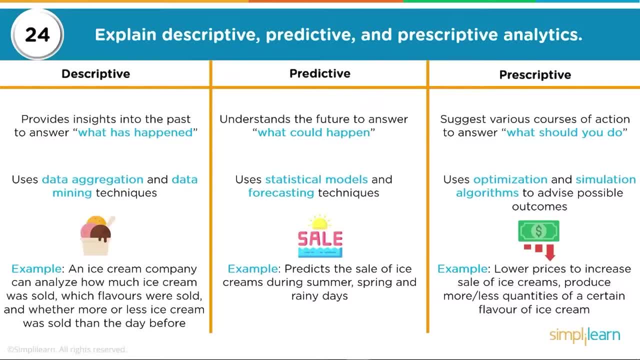 that we're going to need in hospital, that we're going to need in hospital: beds and prescriptive. what can we change? beds and prescriptive? what can we change beds and prescriptive? what can we change in our setup to have a better outcome, in our setup to have a better outcome? 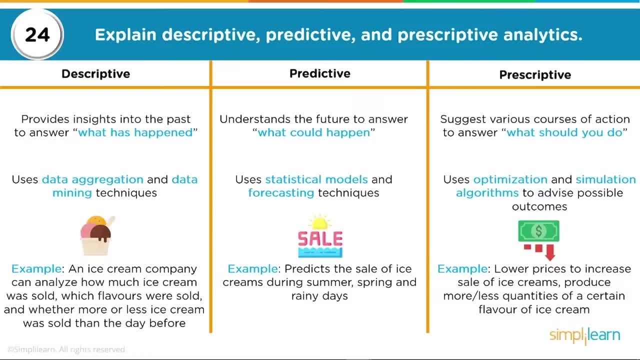 in our setup to have a better outcome. maybe if we did more social distancing. maybe if we did more social distancing, maybe if we did more social distancing if we tracked the virus, if we tracked the virus, if we tracked the virus, how do these different things directly? how do these different things directly? 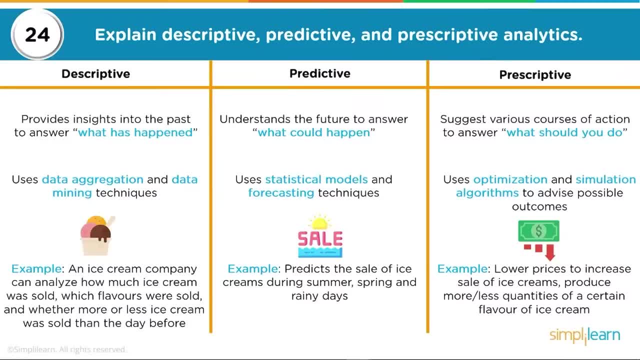 how do these different things directly affect the end and can we create a affect the end? and can we create a affect the end and can we create a better ending by changing some better ending, by changing some better ending, by changing some underlying criteria, underlying criteria, underlying criteria: what are the different types of? 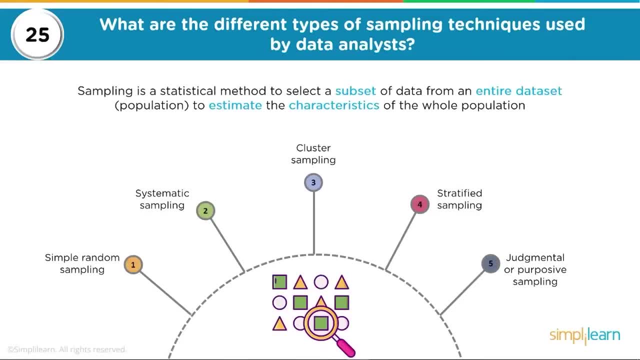 what are the different types of? what are the different types of sampling techniques used by data sampling techniques used by data sampling techniques used by data analysts: analysts- analysts. sampling is a statistical method to sampling is a statistical method to sampling is a statistical method to select a subset of data from an entire. 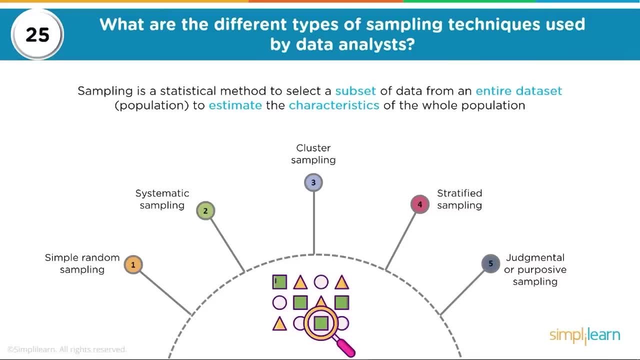 select a subset of data from an entire. select a subset of data from an entire data set: data set: data set population. to estimate the population, to estimate the population, to estimate the characteristics of the whole, characteristics of the whole, characteristics of the whole population. one we can do a simple random. 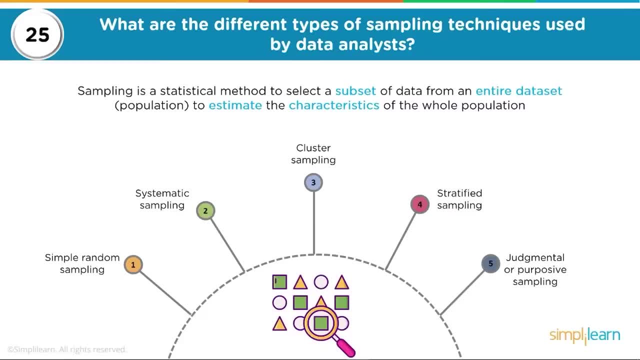 population one. we can do a simple random population one. we can do a simple random sampling so we can just pick out 500 sampling. so we can just pick out 500 sampling. so we can just pick out 500 random people in the united states to random people in the united states to. 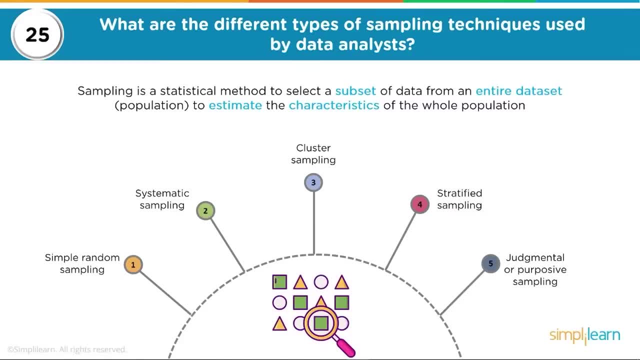 random people in the united states to sample them. they call it a population in sample them. they call it a population in sample them. they call it a population in regular data. we also call that a regular data. we also call that a regular data. we also call that a population, just because that's where it. 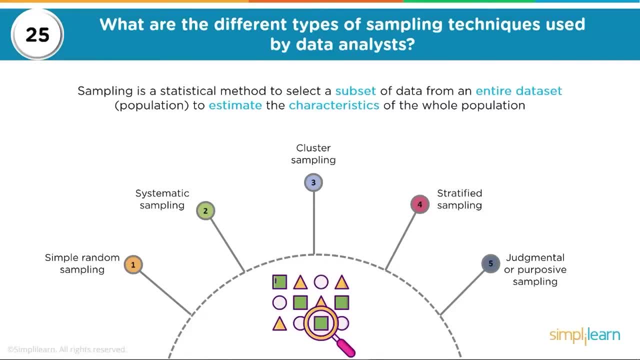 population. just because that's where it population, just because that's where it came from, was mainly from doing census came from. was mainly from doing census came from. was mainly from doing census. systematic sampling- systematic sampling. systematic sampling. cluster sampling. cluster sampling. cluster sampling. stratified sampling- stratified sampling. 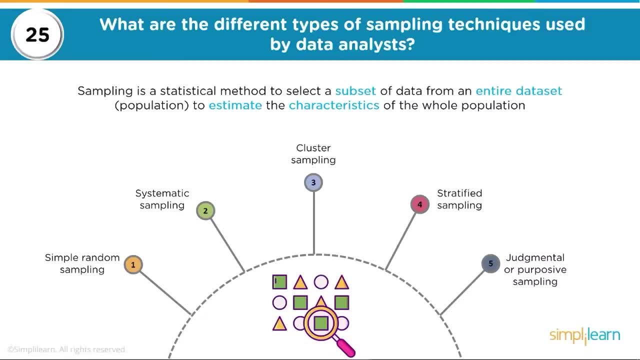 stratified sampling and judgment or purposive sampling and judgment, or purposive sampling and judgment or purposive sampling. then we have our systematic sampling, then we have our systematic sampling, then we have our systematic sampling. that's where you're doing like. that's where you're doing like. 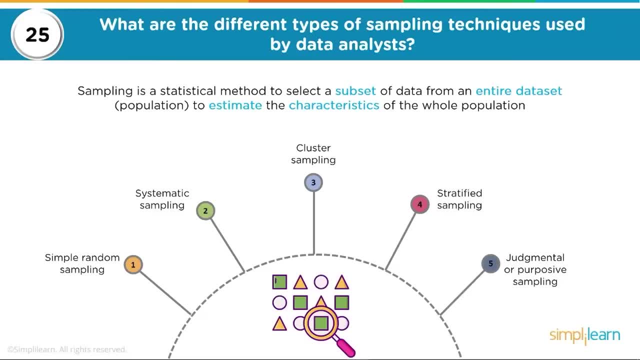 that's where you're doing, like using 1- 5, using 1- 5, using 1- 5, 10, 15- 20. use a very systematic approach. 10- 15- 20. use a very systematic approach: 10- 15- 20. use a very systematic approach for pulling samples. 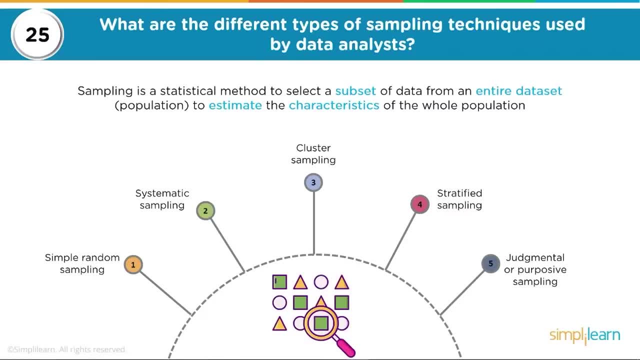 for pulling samples, for pulling samples from the setup cluster, sampling from the setup cluster, sampling from the setup cluster sampling. that's where we look at it. we say hey, that's where we look at it. we say hey, that's where we look at it. we say hey, some of these things, just naturally. 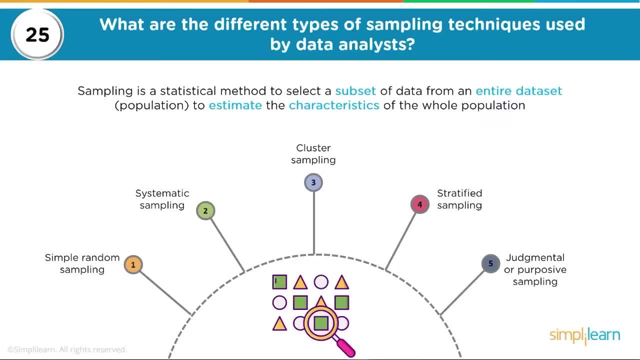 some of these things just naturally. some of these things just naturally grouped together. if you were talking grouped together, if you were talking grouped together, if you were talking about population, which is the really a about population, which is the really a about population, which is the really a nice way of looking at this cluster. 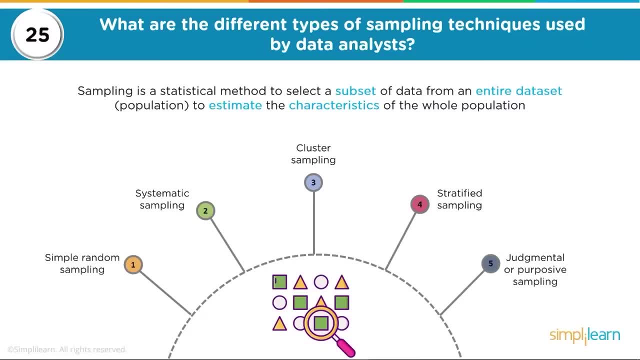 nice way of looking at this cluster. nice way of looking at this cluster. sampling would be: maybe by a zip code. sampling would be maybe by a zip code. sampling would be: maybe by a zip code. we're going to do everybody's zip code. we're going to do everybody's zip code. 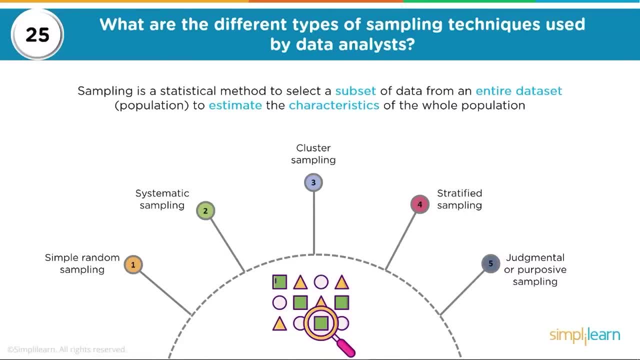 we're going to do everybody's zip code and just naturally cluster it that way and just naturally cluster it that way and just naturally cluster it that way. stratified sampling would be more. stratified sampling would be more. stratified sampling would be more. looking for shared things. the group has 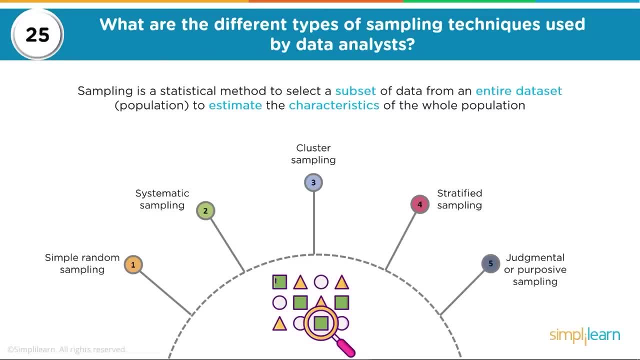 looking for shared things. the group has looking for shared things. the group has: like income, like income, like income. so if you're studying something on, so, if you're studying something on, so, if you're studying something on poverty, you might look at their poverty. you might look at their. 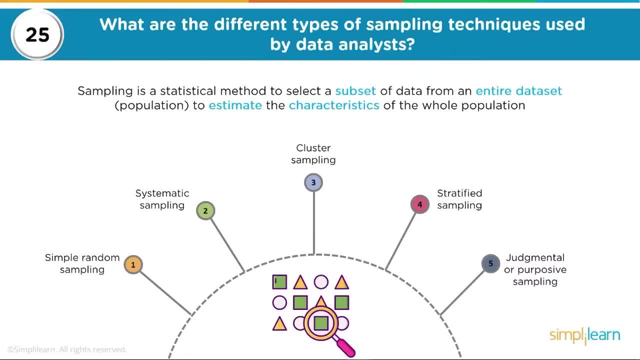 poverty. you might look at their naturally group people, naturally group people, naturally group people, based on income to begin with and then based on income to begin with and then based on income to begin with, and then study those individuals in the income to study those individuals in the income to 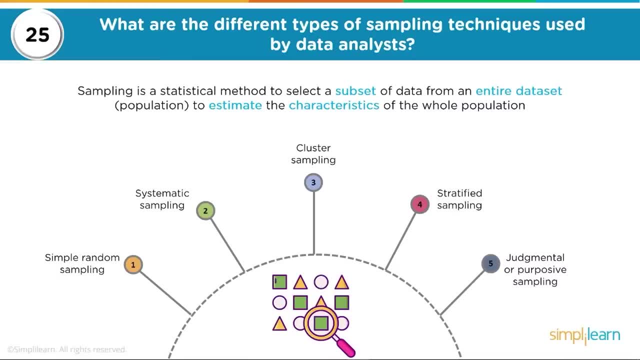 study those individuals in the income to find out, find out, find out what kind of traits they have, what kind of traits they have, what kind of traits they have, and then judgmental and then judgmental and then judgmental that is. that is, that is where the 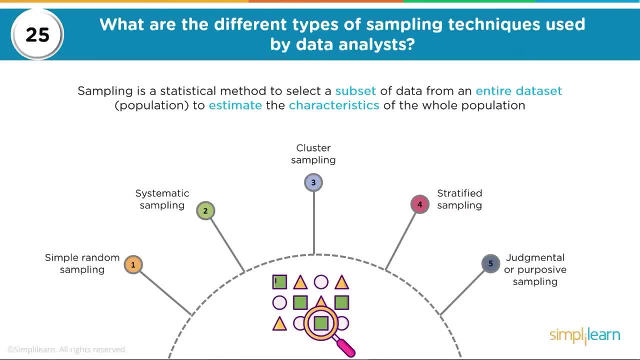 That's where we look at it. We say, hey, some of these things just naturally group together. if you were talking about population- Which is the really a nice way of looking at this- cluster sampling would be maybe by zip code. We're going to do everybody's zip code and just naturally cluster it that way. 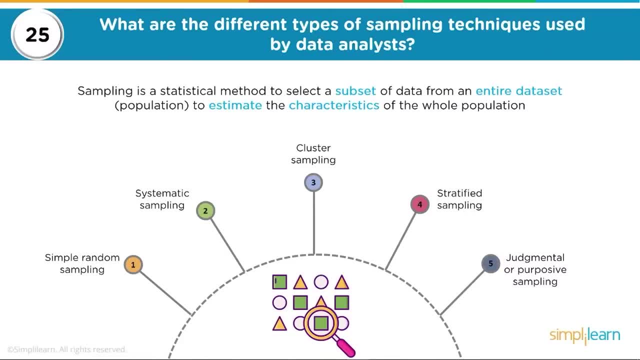 Stratified sampling would be more looking for shared things. a group has like income, So if you're studying something on poverty, you might look at their- naturally group people Based on income to begin with and then study those individuals in the income to find out what kind of traits they have. 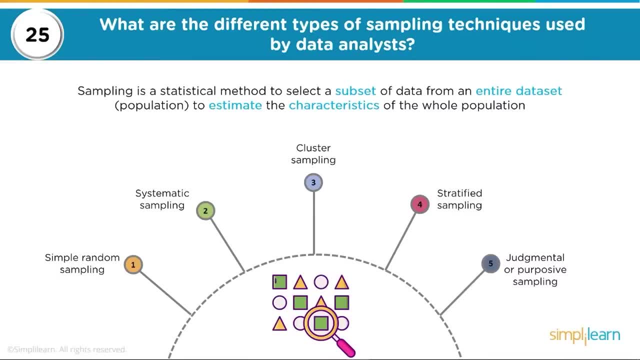 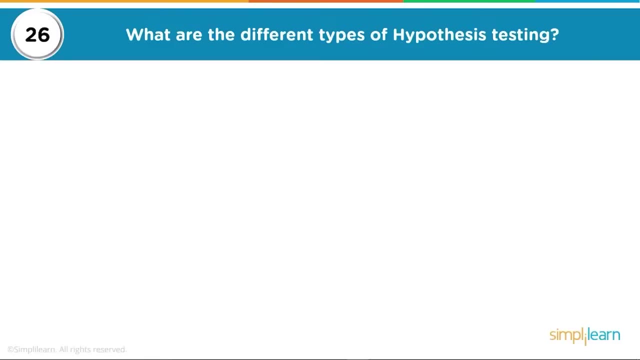 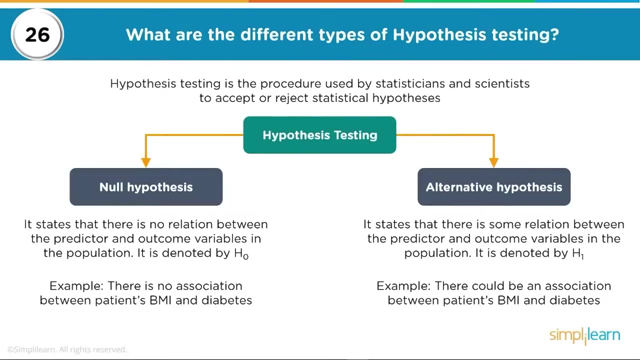 and then judgmental. that is where the researcher very carefully selects each member of their own group, So it's very much based on their personal knowledge. Jumping on the 26.. What are the different types of hypothesis testing? Hypothesis testing is a procedure used by statisticians and scientists to 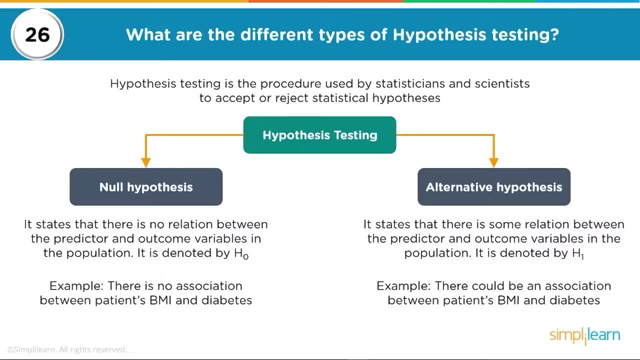 Accept or reject statistical hypothesis. We start with a hypothesis testing. We have no hypothesis and alternative hypothesis on the null hypothesis. it states that there is no relation between the predictor and the outcome variables in the population. it is denoted by H naught Example. there is no association between patients. 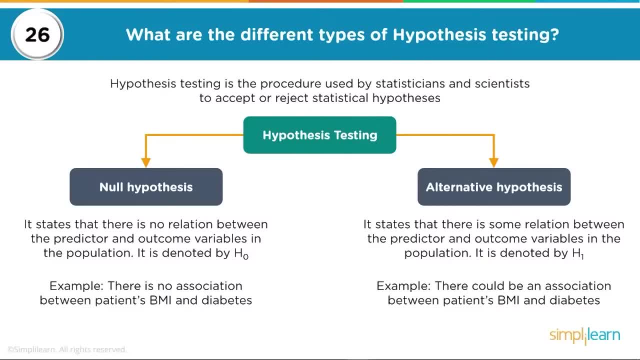 BMI and diabetes. alternative hypothesis: it states there is some relation between the predictor and outcome variables in the population. It is denoted by H1 Example. there could be an association between patients BMI and diabetes. And that's the body mass index. if you didn't catch the BMI. 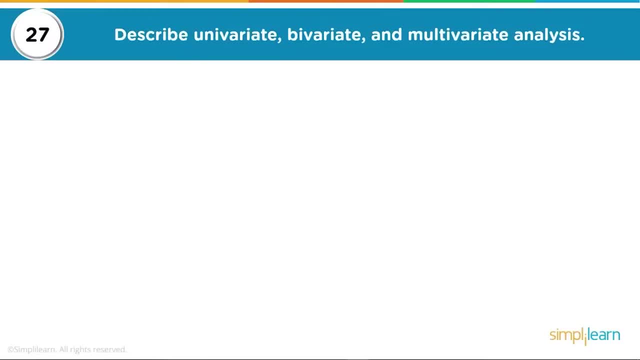 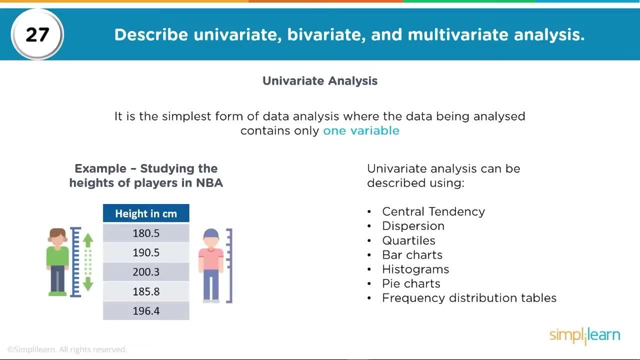 And you're not in medical- describe univariate, bivariate and multivariate analysis. a Univariate analysis: it is the simplest form of data analysis, where the data being analyzed contains only one variable. An example is studying the heights of players in the NBA. Because it's so simple, it can be described using central tendencies. 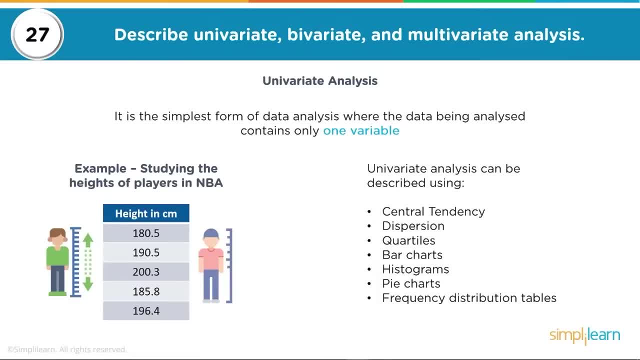 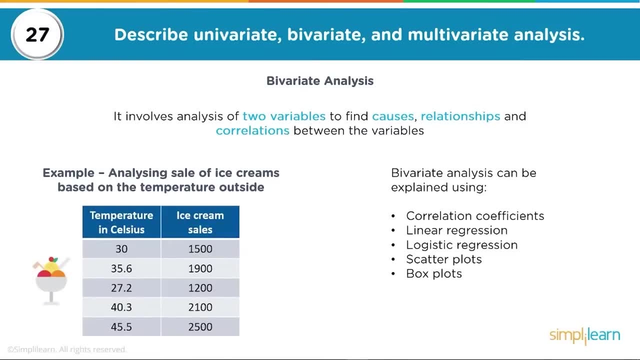 dispersion quartiles, bar charts, histograms, pie charts, frequency distribution tables. The bivariate analysis: it involves analysis of two variables to find causes, relationships and correlations between the variables. Example: analyzing sale of ice creams based on the temperature outside. Bivariate analysis can be explained using correlation coefficients, linear regression. 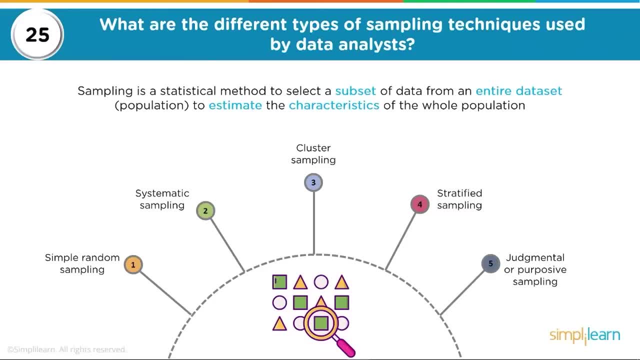 where the, where the researcher very carefully selects, each researcher very carefully selects, each researcher very carefully selects each member of their own group, member of their own group, member of their own group. so it's very much so, it's very much so, it's very much based on their personal knowledge. 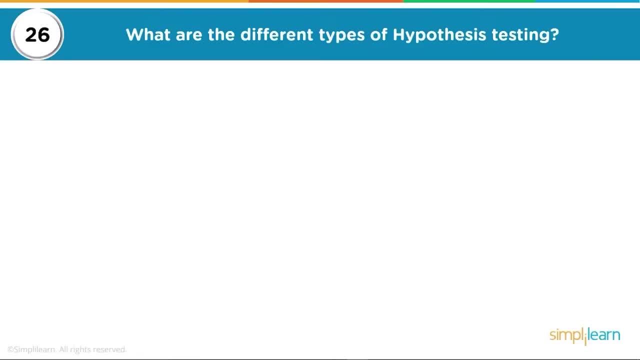 based on their personal knowledge. based on their personal knowledge. jumping on the 26. what are the different? jumping on the 26. what are the different? jumping on the 26. what are the different types of hypothesis testing? types of hypothesis testing. types of hypothesis testing. hypothesis testing is a procedure used. 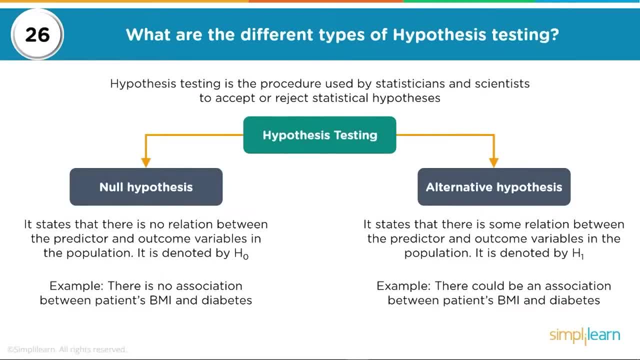 hypothesis testing is a procedure used. hypothesis testing is a procedure used by statisticians and scientists to by statisticians and scientists to by statisticians and scientists to accept or reject statistical hypothesis. accept or reject statistical hypothesis. accept or reject statistical hypothesis. we start with the hypothesis testing. we 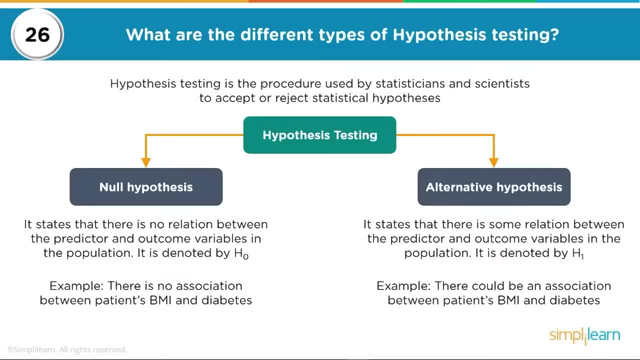 we start with the hypothesis testing. we we start with the hypothesis testing. we have null hypothesis and alternative. have null hypothesis and alternative. have null hypothesis and alternative hypothesis: hypothesis: hypothesis on the null hypothesis. it states that on the null hypothesis. it states that on the null hypothesis. it states that there is no relation between the. 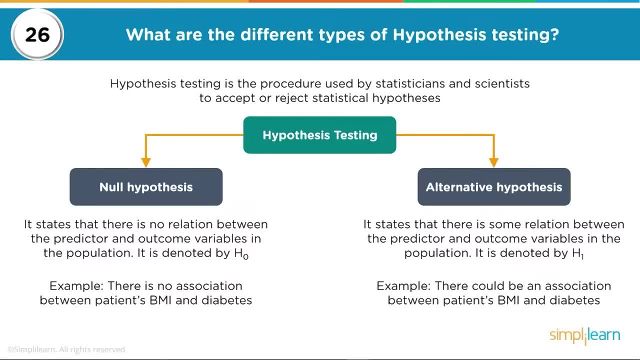 there is no relation between the. there is no relation between the predictor and the outcome variables in predictor and the outcome variables in predictor and the outcome variables in the population. it is denoted by h0 the population. it is denoted by h0 the population. it is denoted by h0, example. there is no association between 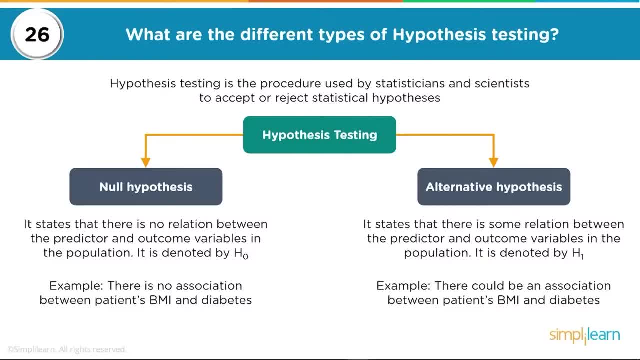 example, there is no association between example, there is no association between patients: bmi and diabetes patients, bmi and diabetes patients, bmi and diabetes. alternative hypothesis. it states there alternative hypothesis. it states there alternative hypothesis. it states there is some relation between the predictor. is some relation between the predictor? 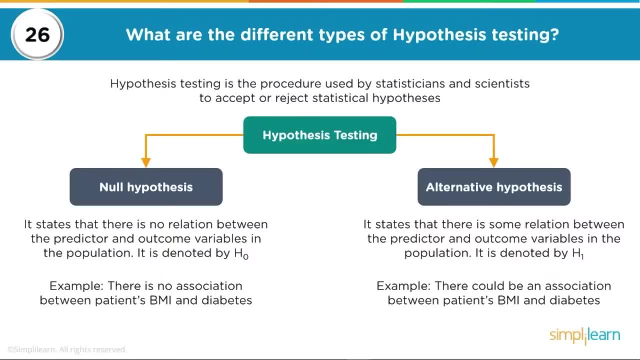 is some relation between the predictor and outcome variables in the population and outcome variables in the population and outcome variables in the population. it is denoted by h1 example there could. it is denoted by h1 example there could. it is denoted by h1 example. there could be an association between patients bmi. 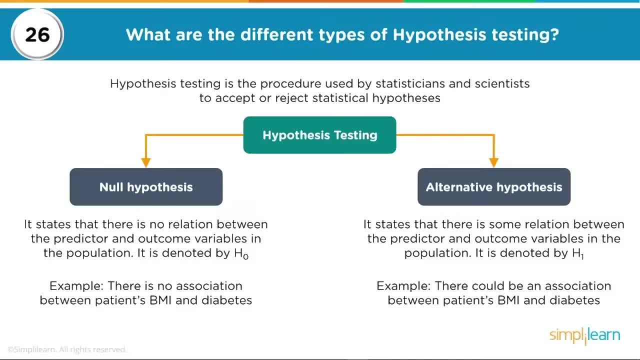 be an association between patients, bmi and diabetes, and that's the body mass and diabetes, and that's the body mass and diabetes and that's the body mass index. if you didn't catch the bmi and index, if you didn't catch the bmi and index, if you didn't catch the bmi and you're not medical. 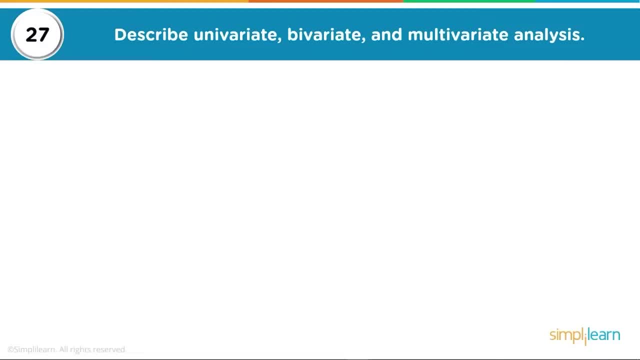 you're not medical. you're not medical. describe univariate bivariate. and describe univariate bivariate. and describe univariate, bivariate and multivariate analysis. multivariate analysis, multivariate analysis, a univariate analysis- it is the simplest. a univariate analysis- it is the simplest. 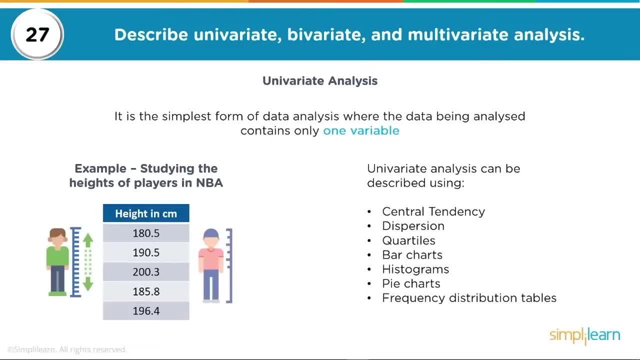 a univariate analysis. it is the simplest form of data analysis, where the data form of data analysis, where the data form of data analysis, where the data being analyzed contains only one being analyzed contains only one being analyzed contains only one variable. an example of studying the variable. an example of studying the 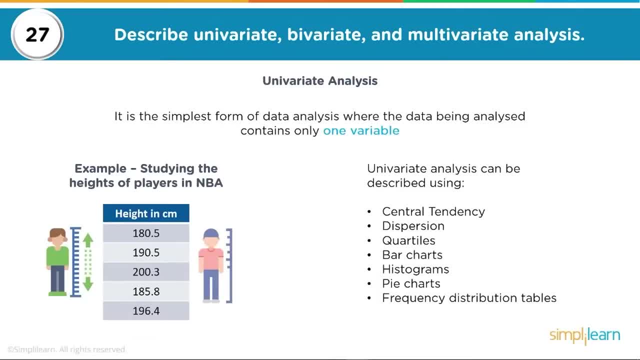 variable an example of studying the heights of players in the nba. heights of players in the nba. heights of players in the nba. because it's so simple it can be. because it's so simple it can be. because it's so simple it can be described using central tendencies. 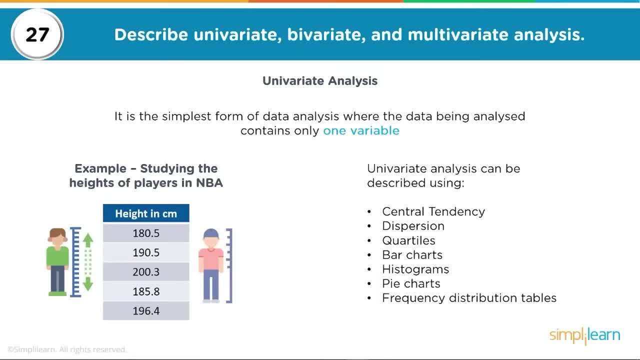 described using central tendencies. described using central tendencies. dispersion quartiles- bar charts. dispersion quartiles- bar charts. dispersion quartiles- bar charts. histograms- pie charts- frequency histograms- pie charts. frequency histograms- pie charts- frequency distribution tables- distribution tables. distribution tables. the bivariate analysis. it involves the bivariate analysis. it involves: 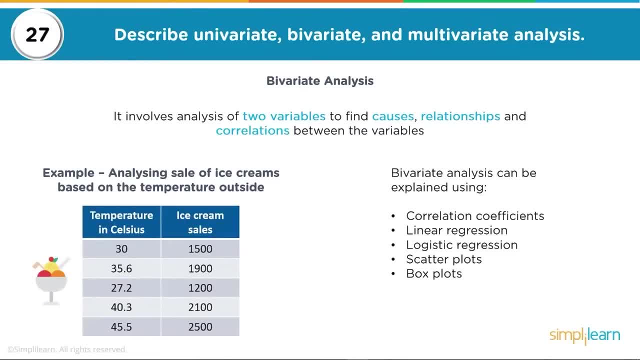 the bivariate analysis. it involves: analysis of two variables to find causes. analysis of two variables to find causes. analysis of two variables to find causes, relationships and correlations between relationships and correlations between relationships and correlations between the variables. example: analyzing sale of the variables. example: analyzing sale of. 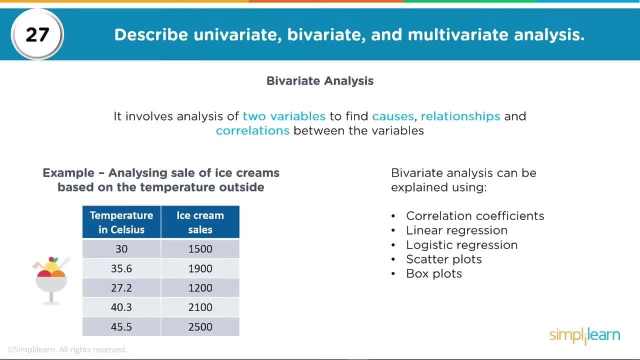 the variables. example: analyzing sale of ice creams based on the temperature. ice creams based on the temperature. ice creams based on the temperature outside, outside outside. bivariate analysis can be explained using bivariate analysis can be explained using bivariate analysis can be explained using correlation coefficients: linear. 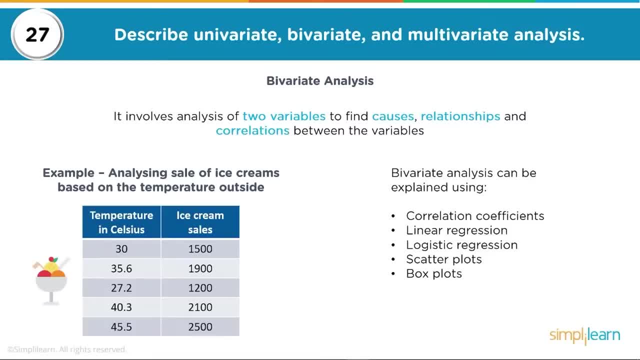 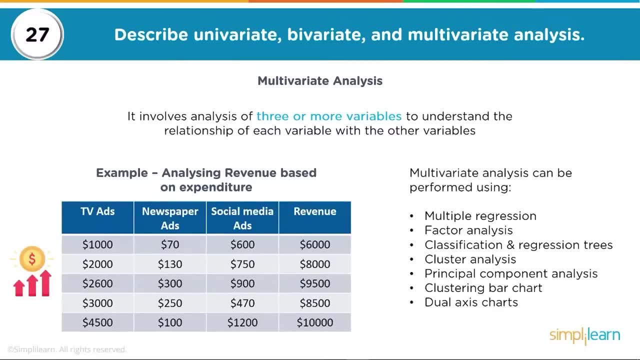 correlation coefficients- linear correlation coefficients- linear regression, regression regression, logistic regression, scatter plots- logistic regression, scatter plots, logistic regression, scatter plots and box plots and box plots and box plots and multivariate analysis. it involves and multivariate analysis. it involves and multivariate analysis. it involves analysis, analysis, analysis of three or more variables to understand. 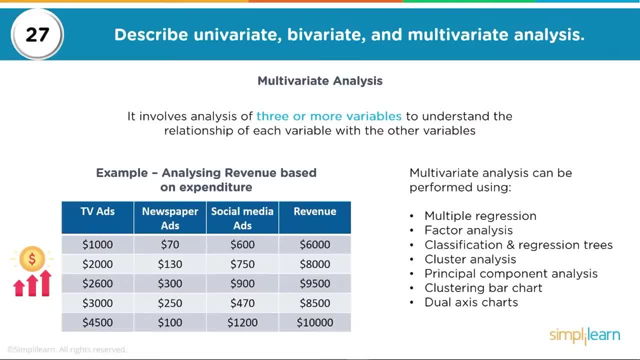 of three or more variables. to understand of three or more variables. to understand the relationship of each variable, the relationship of each variable, the relationship of each variable with the other variables. example with the other variables. example with the other variables. example: analyzing revenue based on expenditure. analyzing revenue based on expenditure. 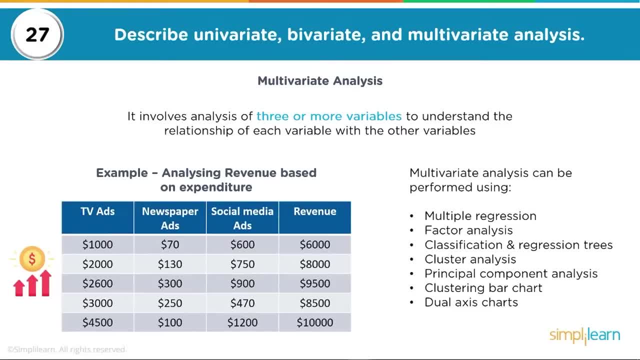 analyzing revenue based on expenditure. so if we have our tv ads, we have our. so if we have our tv ads, we have our. so if we have our tv ads, we have our newspaper ads or social media ads, newspaper ads or social media ads, newspaper ads or social media ads and a revenue. we can now compare all. 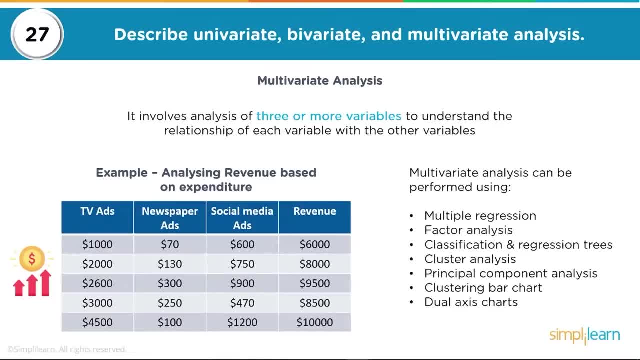 and a revenue. we can now compare all and a revenue. we can now compare all. those together, those together, those together, the multiverte analysis can be performed. the multiverte analysis can be performed. the multiverte analysis can be performed using multiple regression. using multiple regression. 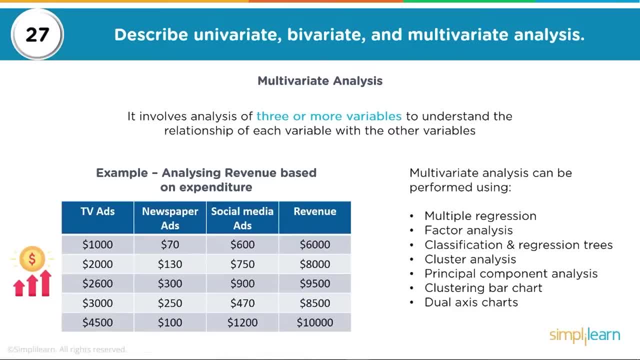 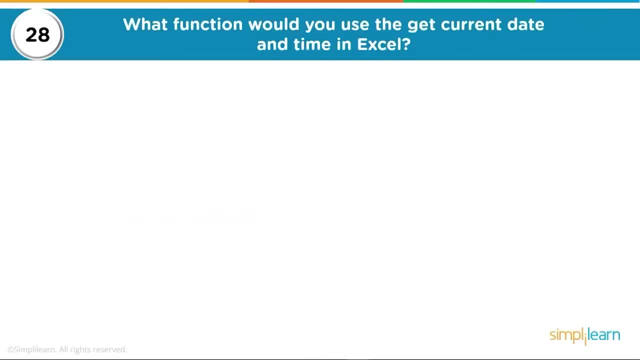 using multiple regression: factor analysis. classification and factor analysis. classification and factor analysis. classification and regression trees- cluster analysis. regression trees- cluster analysis. regression trees- cluster analysis. principal component analysis- clustering- principal component analysis- clustering- principal component analysis. clustering bar chart. bar chart- bar chart- dual axis chart. what function would you? 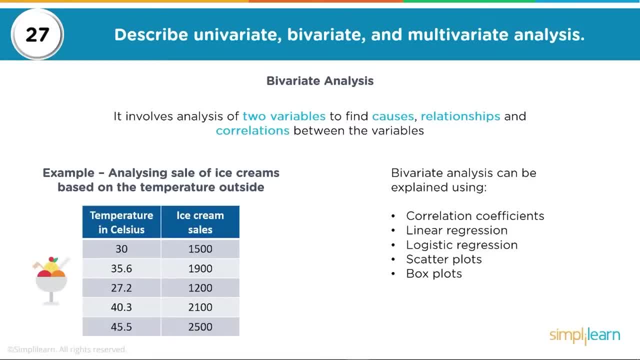 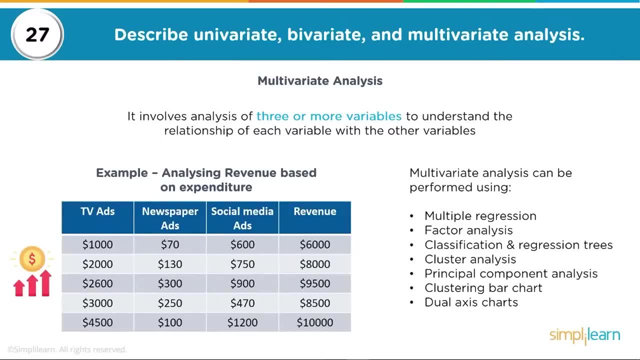 logistic regression, scatter plots and box plots, and And multivariate analysis. it involves analysis of three or more variables to understand the relationship of each variable with the other variables. Example: analyzing revenue based on expenditure. So if we have our TV ads, we have our newspaper ads or social media ads and a revenue. 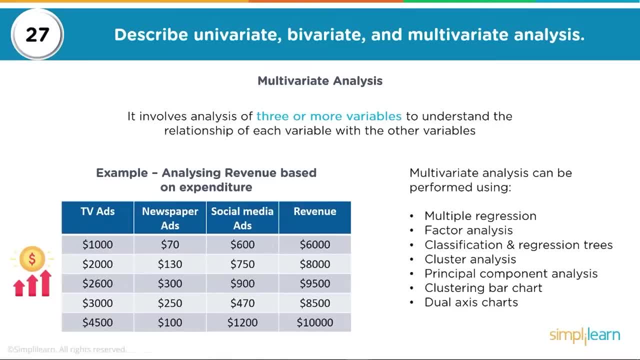 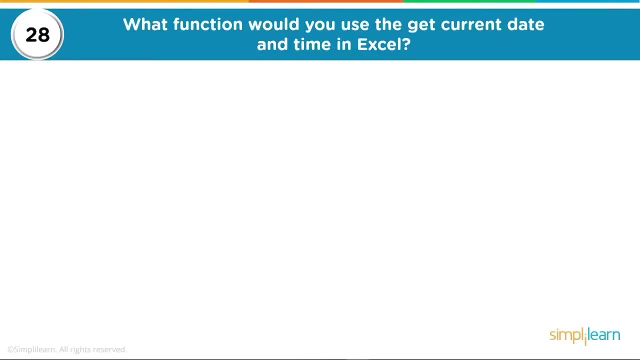 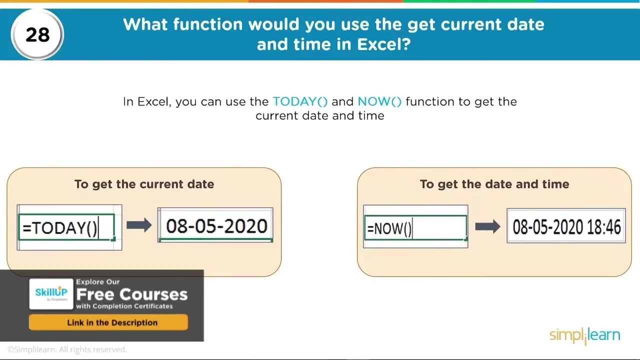 We can now compare all those together. the multivariate analysis can be performed using multiple regression: factor analysis, classification and regression trees. cluster analysis, principal component analysis, clustering bar chart, dual axis chart. What function would you use to get the current date and time in Excel? in Excel, you can use the today and now function to get the current date and time. 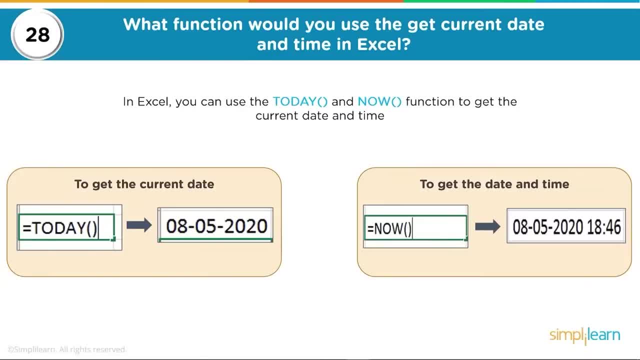 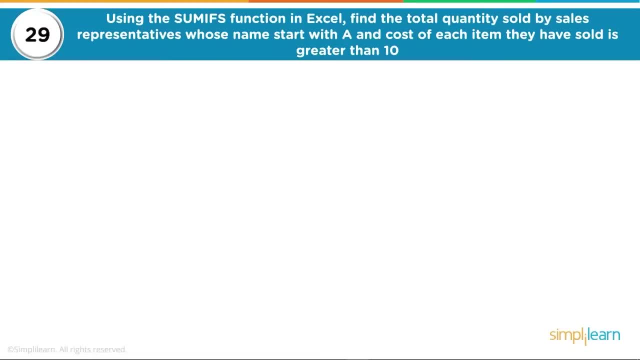 You can see down here with the two examples. We're just equals today or equals now. using the sum ifs function in Excel, find the total Quantity sold by sales Representatives whose names start with a and the cost of each item they have sold is greater than 10. 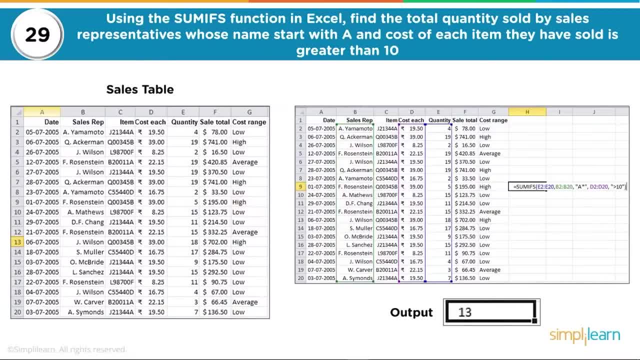 And you can see, here on the left We have our actual table and Then we want to go ahead and sum ifs. so we want the e2 through e20, b2 through b20, Greater than 10, and this basically is just saying, hey, we're going to take everything in the e column. 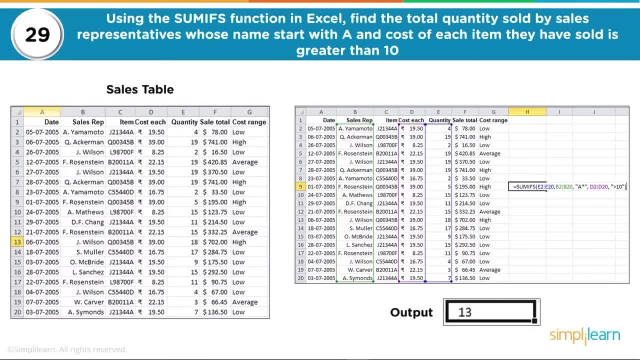 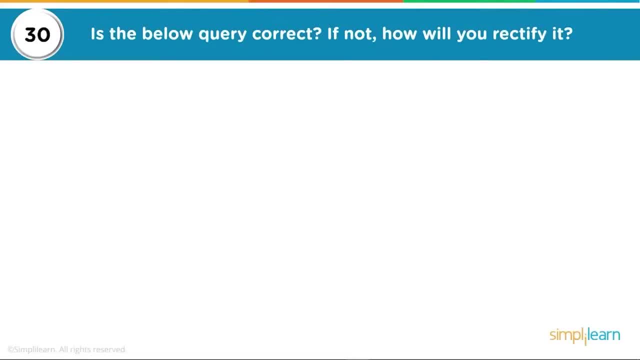 And we're going to sum it up- but only those objects where the d column is greater than 10.. That's what that means there. Is the below query correct? if not, how will you rectify it? Select customer ID: year, order date as order year from order. 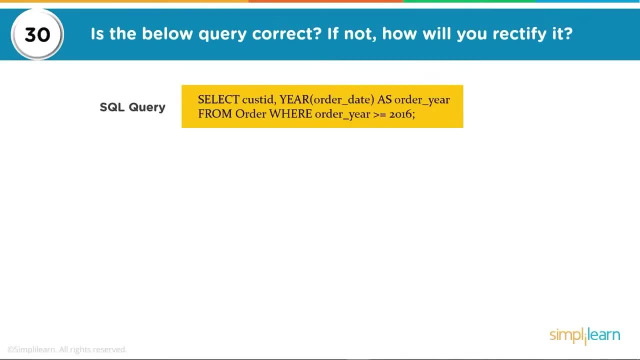 Where order year is greater than or equal to 2016, And hopefully you caught it right there. It's in the devil's in the details. We can't not to use the alias name while filtering data using the WHERE clause, So the correct format is all the same, except for where it says WHERE the year order date. 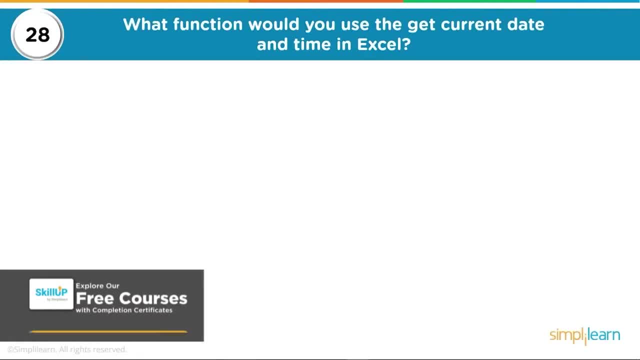 dual axis chart. what function would you dual axis chart? what function would you use to get the current date and time in use? to get the current date and time in use. to get the current date and time in excel, excel, excel. in excel, you can use the today and now. 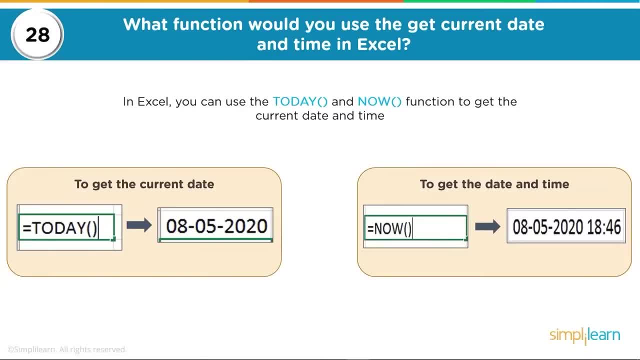 in excel you can use the today and now. in excel you can use the today and now function to get the current date and function to get the current date and function to get the current date and time time time. you can see down here with the two. you can see down here with the two. 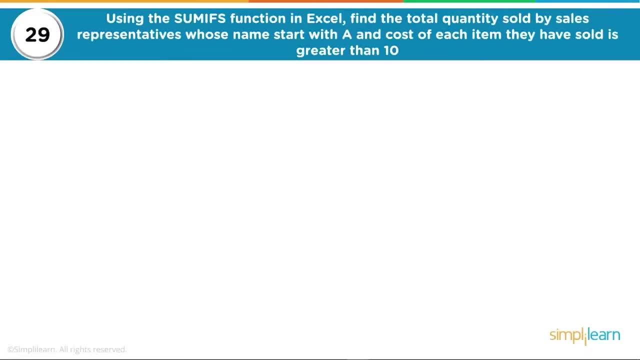 you can see down here with the two examples: we're just equals today. or examples: we're just equals today. or examples: we're just equals today or equals now. equals now. equals now. using the sum ifs function in excel. using the sum ifs function in excel, using the sum ifs function in excel, find the total quantity sold by sales. 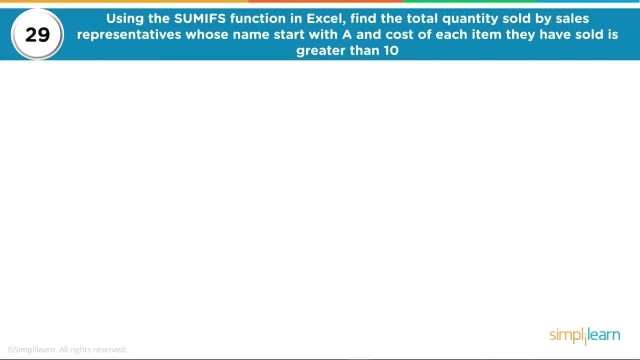 find the total quantity sold by sales. find the total quantity sold by sales representatives: representatives- representatives whose names start with a and the cost of whose names start with a. and the cost of whose names start with a and the cost of each item they have sold is greater than. 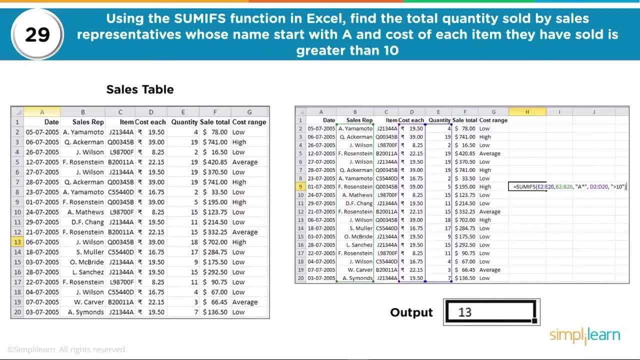 each item they have sold is greater than each item they have sold is greater than 10.. 10.. 10. and you can see here on the left we have, and you can see here on the left we have, and you can see here on the left we have our actual table. 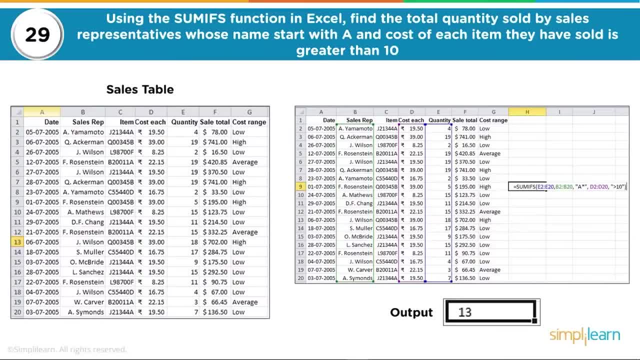 our actual table, our actual table. and then we want to go ahead and sum ifs, and then we want to go ahead and sum ifs, and then we want to go ahead and sum ifs. so we want the e2 through e20, so we want the e2 through e20. 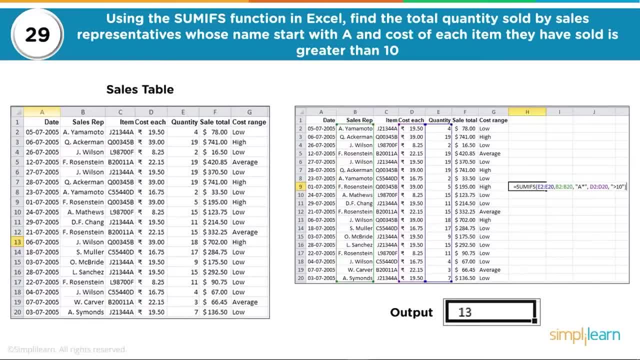 so we want the e2 through e20, b2 through b20 greater than 10.. b2 through b20 greater than 10.. b2 through b20 greater than 10.. and this basically is just saying hey, and this basically is just saying hey. 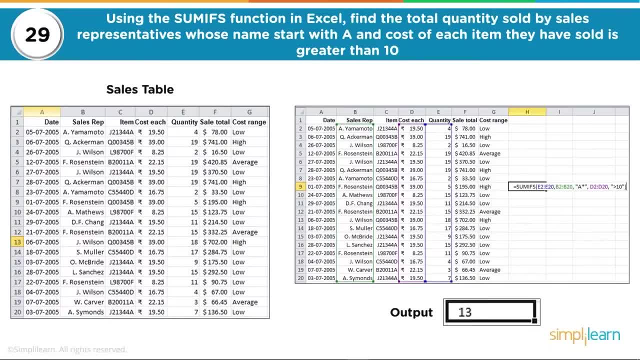 and this, basically, is just saying: hey, we're going to take everything, we're going to take everything, we're going to take everything in the e column and we're going to sum in the e column and we're going to sum in the e column and we're going to sum it up, but only those. 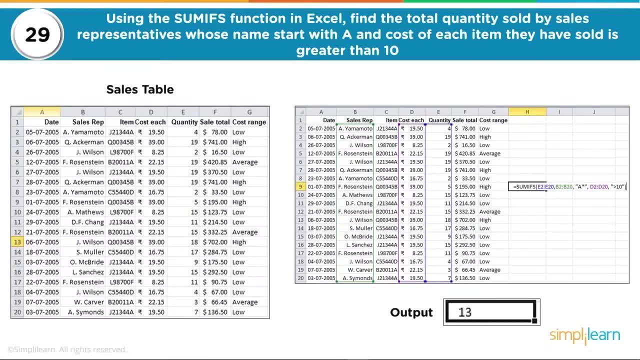 it up, but only those it up, but only those objects where the d column is greater than objects where the d column is greater than objects where the d column is greater than 10. that's what that means there 10. that's what that means. there 10. that's what that means there. is the below query correct? if not, how? 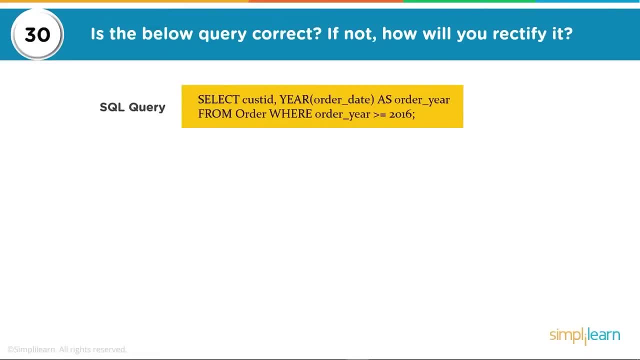 is the below query correct? if not, how is the below query correct? if not, how will you rectify it? will you rectify it? will you rectify it? select customer id year order date: as select customer id year order date: as select customer id year order date: as order year from order. 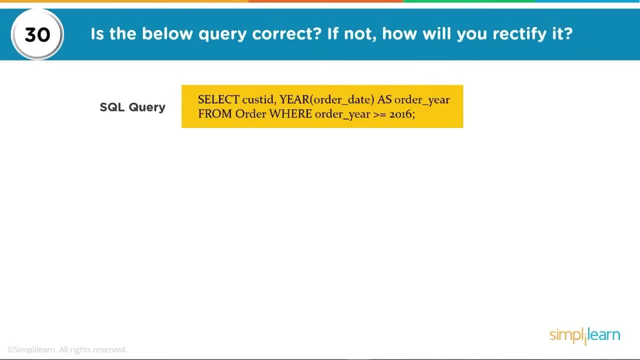 order year from order. order year from order where order year is greater than: or where order year is greater than, or where order year is greater than or equal to 2016.. equal to 2016.. equal to 2016.. and hopefully you caught it right there. 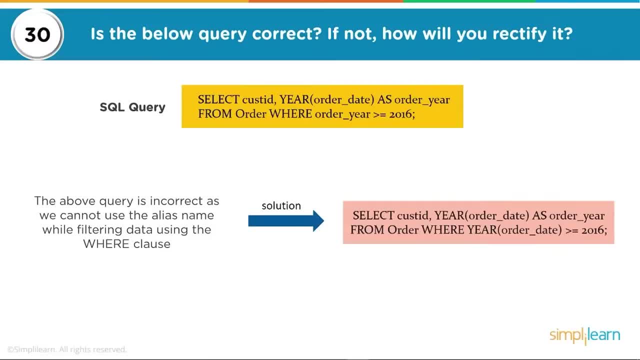 and hopefully you caught it right there. and hopefully you caught it right there. uh, it's in the devil's in the details. uh, it's in the devil's in the details. uh, it's in the devil's in the details. we can't not use the alias name while. 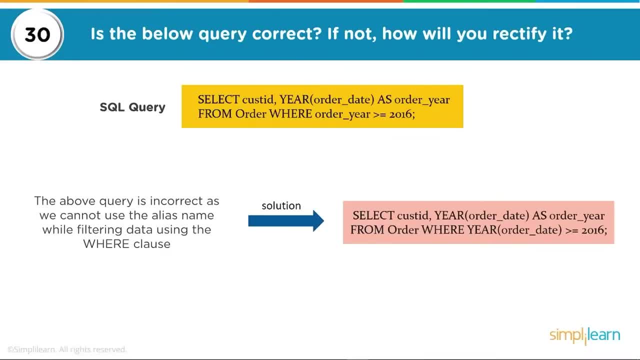 we can't not use the alias name. while. we can't not use the alias name while filtering data using the where clause. filtering data using the where clause. filtering data using the where clause. so the correct format is all the same. so, the correct format is all the same. 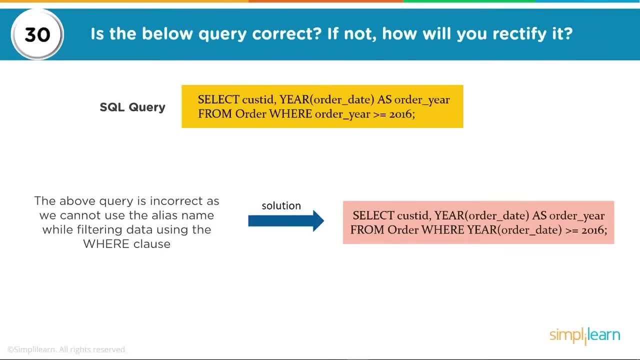 so the correct format is all the same, except for where it says where. except for where it says where. except for where it says where the year, the year, the year order date is greater than or equal to 16. order date is greater than or equal to 16. 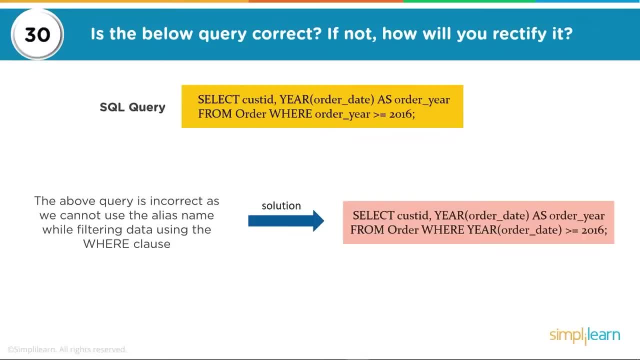 order date is greater than or equal to 16, versus using the order year which we, versus using the order year which we, versus using the order year which we assign under the select setup. assign under the select setup. assign under the select setup. how are union intersect and accept used? 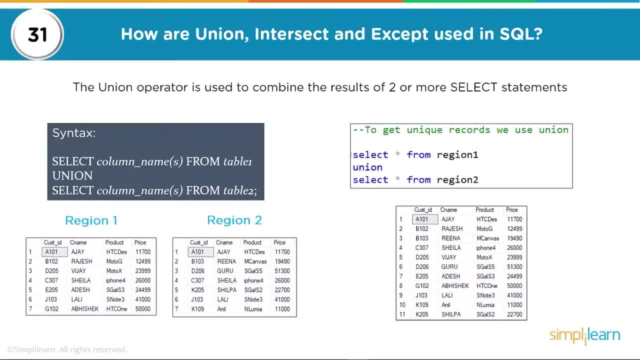 how are union intersect and accept used? how are union intersect and accept used in sql, in sql? in sql, the union operator is used to combine the. the union operator is used to combine the. the union operator is used to combine the results of two or more select. results of two or more select. 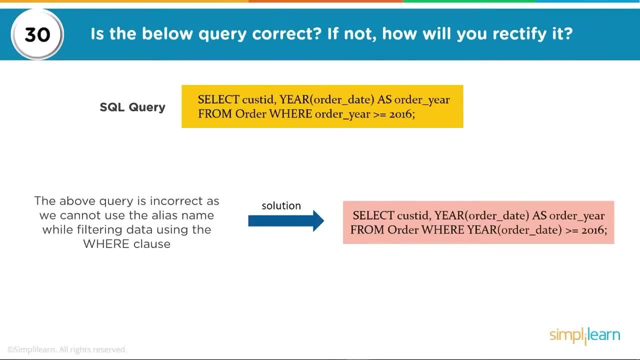 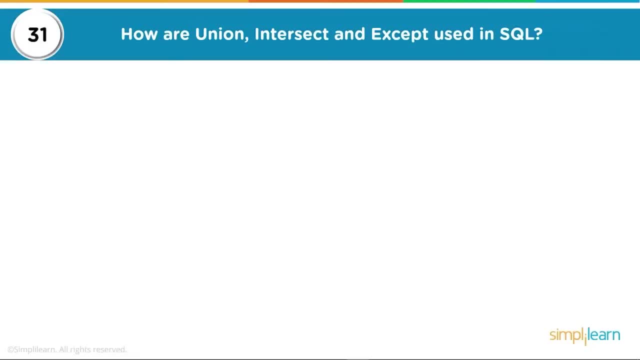 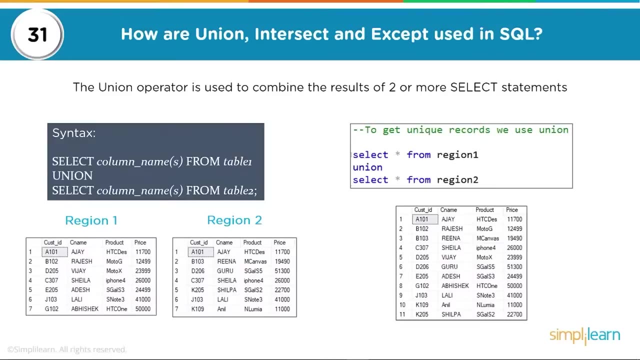 is greater than or equal to 16, versus using the order year which we assign under the SELECT setup. How are UNION, INTERSECT and ACCEPT used in SQL? The UNION operator is used to combine the results of two or more SELECT statements. 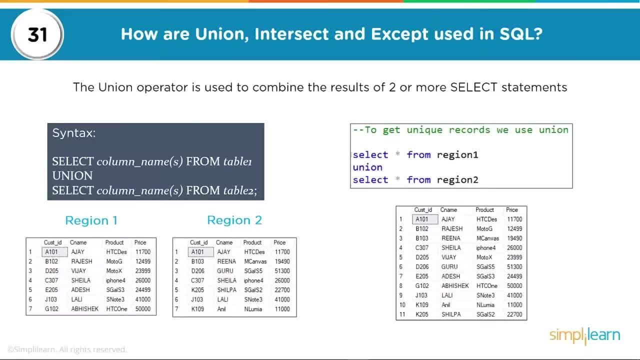 results of two or more select statements, statements, statements, and you can see, here we have select star and you can see, here we have select star. and you can see, here we have select star from region one and we're going to make a from region one and we're going to make a. 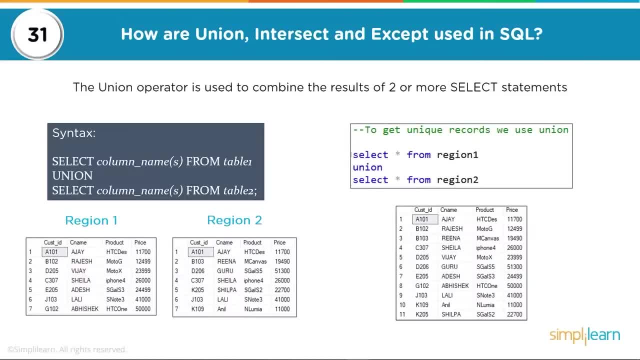 from region one and we're going to make a union with select star from region two, union with select star from region two, union with select star from region two, and it basically takes both these sql and it basically takes both these sql and it basically takes both these sql tables and combines them to form a full 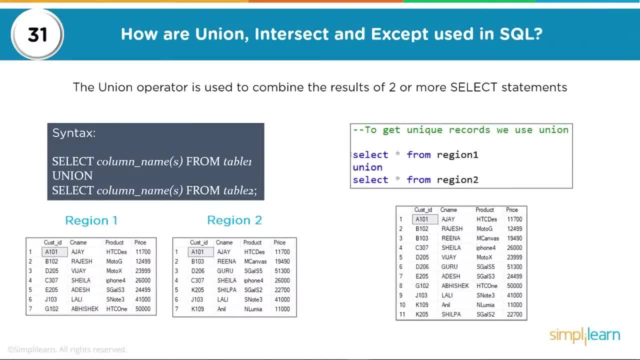 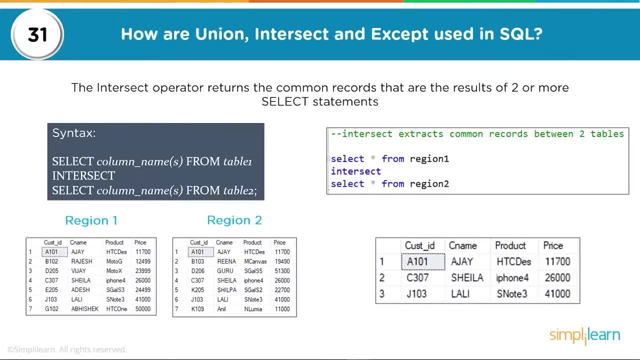 tables and combines them to form a full tables and combines them to form a full new table on there, new table on there, new table on there. so that's your union as we bring. so that's your union as we bring. so that's your union as we bring. one intersect select star from region two. 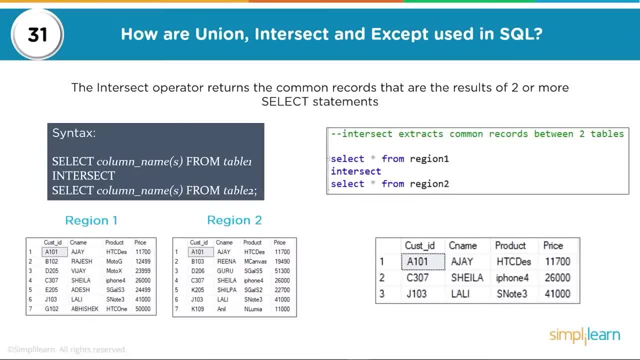 one intersect select star from region two. one intersect select star from region two, and we come up with only those records, and we come up with only those records, and we come up with only those records that are shared, that have the same data, that are shared, that have the same data. 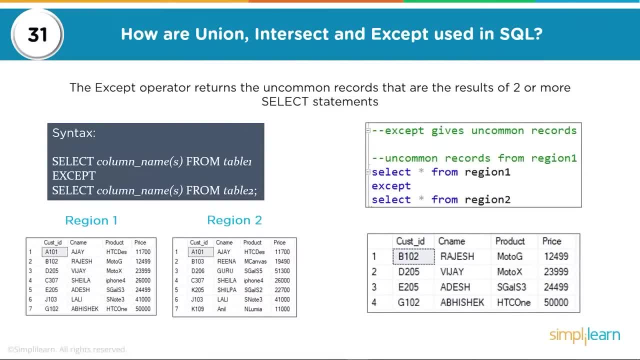 that are shared, that have the same data in them, in them, in them. and hopefully you jumped ahead to the and hopefully you jumped ahead to the and hopefully you jumped ahead to the accept. the accept operator returns the accept. the accept operator returns the accept. the accept operator returns the uncommon records that are the result of. 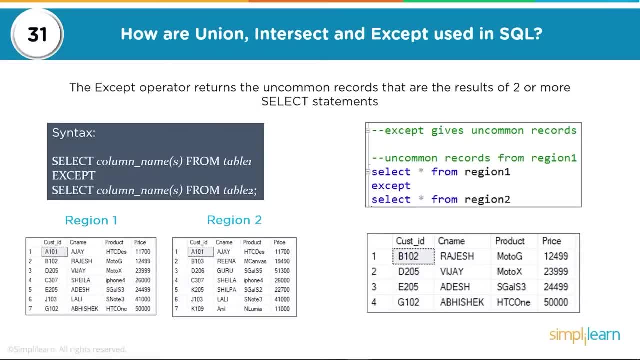 uncommon records that are the result of uncommon records that are the result of two or more select statements. so these two or more select statements, so these two or more select statements, so these are the two records or the records that are the two records or the records that 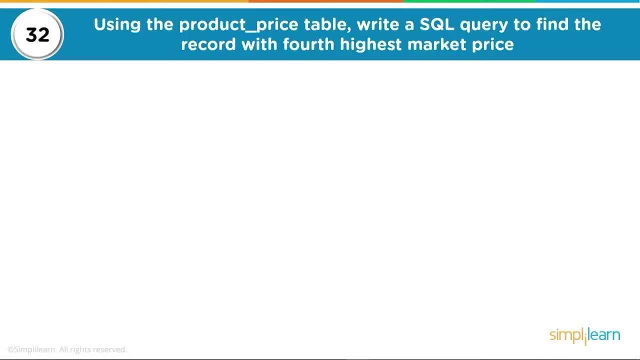 are the two records or the records that are not shared between the two databases? are not shared between the two databases. are not shared between the two databases. using the product price table: write using the product price table. write using the product price table. write an sql query to find the record with the. 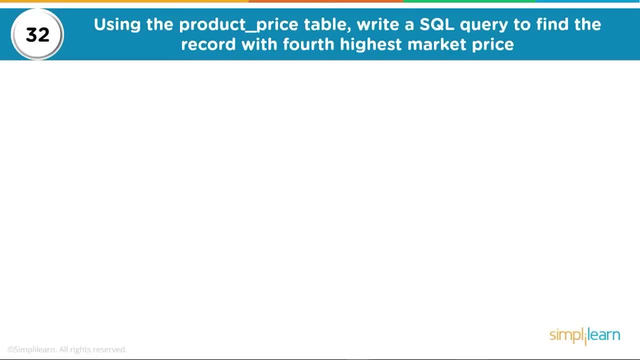 an sql query to find the record with the. an sql query to find the record with the fourth highest, fourth highest, fourth highest market price, market price, market price. so here we have a little bit of a brain. so here we have a little bit of a brain. so here we have a little bit of a brain teaser. 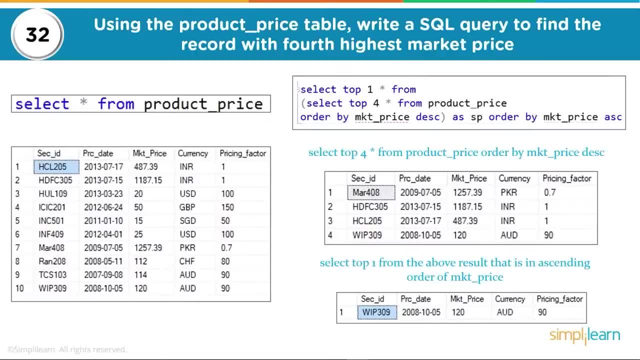 teaser, teaser. they're always fun and the first thing we- they're always fun and the first thing we- they're always fun and the first thing we want to do is we're going to go ahead. want to do is we're going to go ahead. want to do is we're going to go ahead and i'm going to. if you look at the uh. 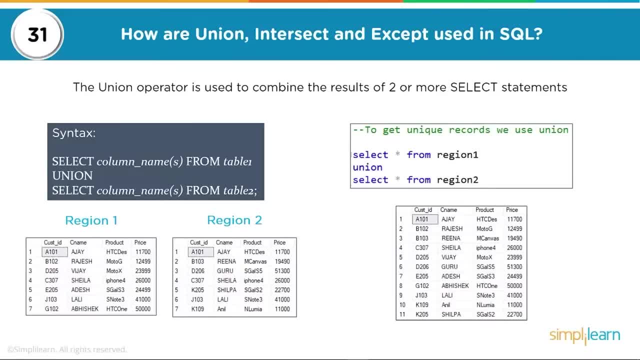 You can see, here we have SELECT star from region 1 and we're going to make a UNION with SELECT star from region 2, and it basically takes both these SQL tables and combines them to form a full new table on there. So that's your UNION as we bring everything together. 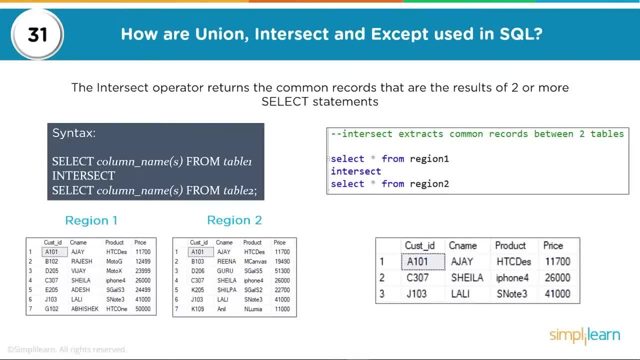 When we look at the INTERSECT operator, it returns the common records that are the result of the two or more SELECT statements. So you can see here we SELECT star from region 1, INTERSECT SELECT star from region 2, and. 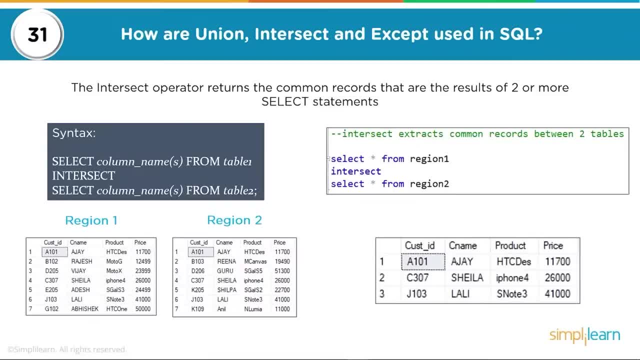 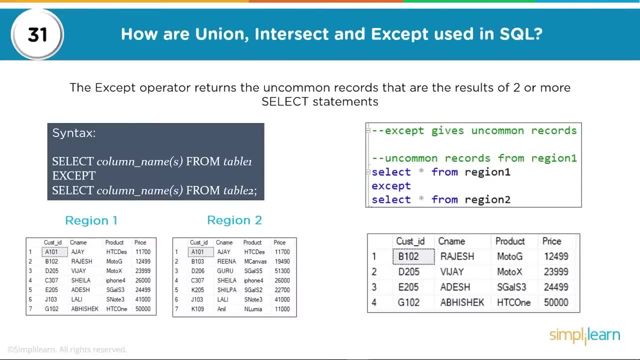 we come up with only those records that are shared, that have the same data in them, And hopefully you jumped ahead to the ACCEPT. The ACCEPT operator returns the uncommon records that are the result of two or more SELECT statements. So these are the two records, or the records that are not shared between the two databases. 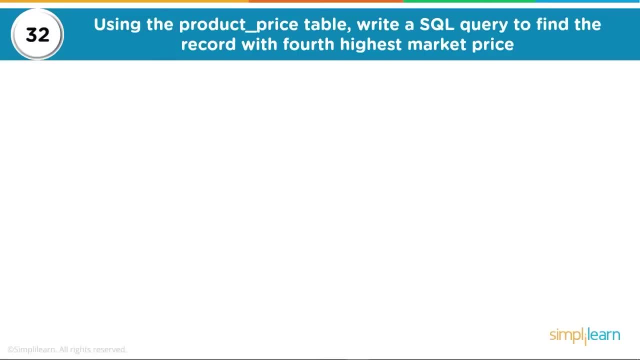 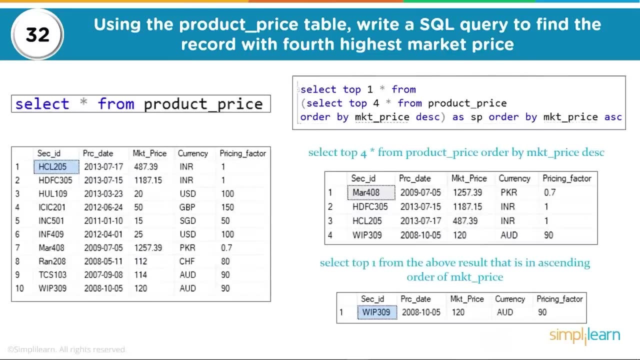 Using the product price table, write an SQL table. This is a simple query to find the record with the fourth highest market price. So here we have a little bit of a brain teaser. They're always fun, And the first thing we want to do is we're going to go ahead, and I'm going to, if you. 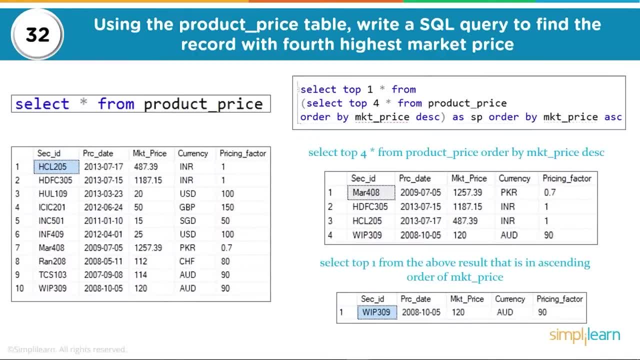 look at the script on the left. we really want the fourth one down. So we're going to select the top four from product price, but we're going to order it by market price descending. SP order by market price ascending. So what we do is we take the top four of the market price ascending and that's going to. 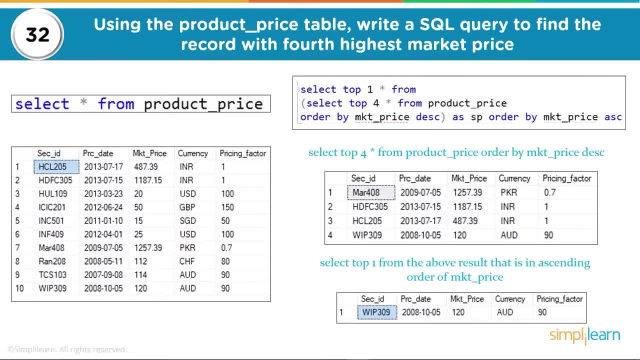 give us the four greatest values, And then we're going to reverse that order and do descending and we're going to take the top one of that, which is going to give us the lowest value, which will be the fourth greatest one in the list. 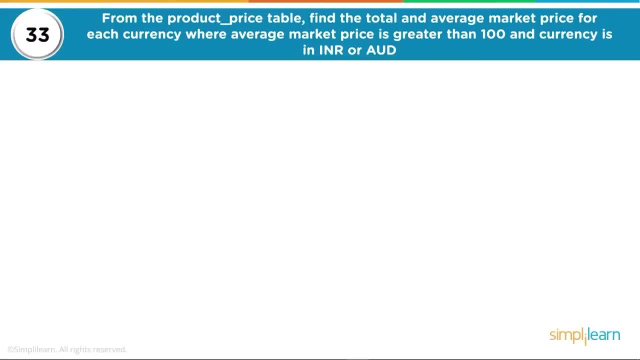 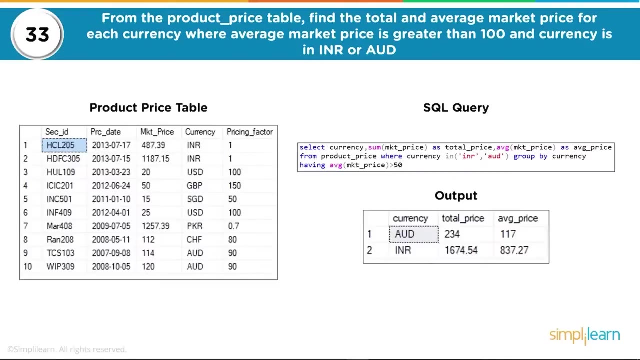 From the product price table find the total and average market price for each currency where the average market price is greater than 100.. And currency is in the INR or the AUD, So INR or AUD, India Rupel or Australia dollar. 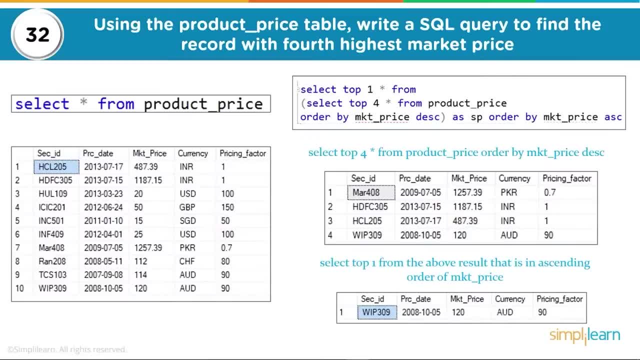 and i'm going to. if you look at the uh and i'm going to. if you look at the uh script on the left script on the left script on the left, we really want the fourth one down. so we really want the fourth one down. so we really want the fourth one down. so we're going to select the top four from. 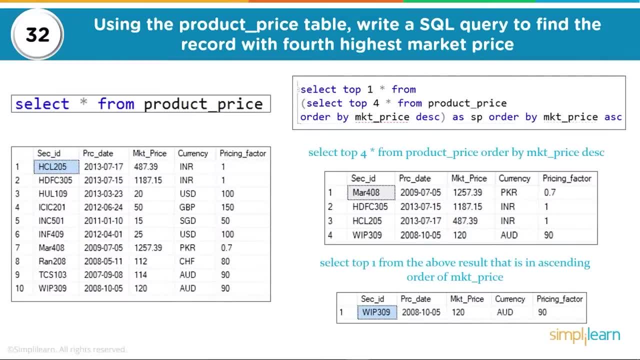 we're going to select the top four from. we're going to select the top four from product price, product price, product price, but we're going to order it by market. but we're going to order it by market. but we're going to order it by market, price descending. 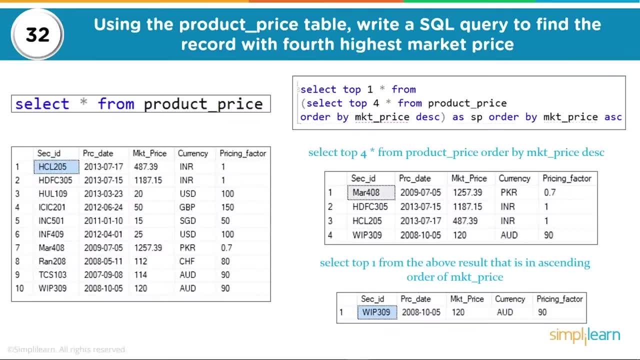 price. descending price descending. sp order by market price ascending. sp order by market price ascending. sp order by market price ascending. so we do. is we take the top, so we do. is we take the top, so we do, is we take the top four of the market price ascending? 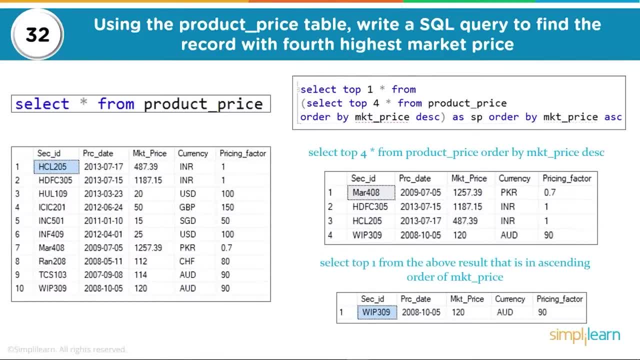 four of the market price ascending, four of the market price ascending, and that's going to give us the four, and that's going to give us the four, and that's going to give us the four greatest values, greatest values, greatest values. and then we're going to reverse that. 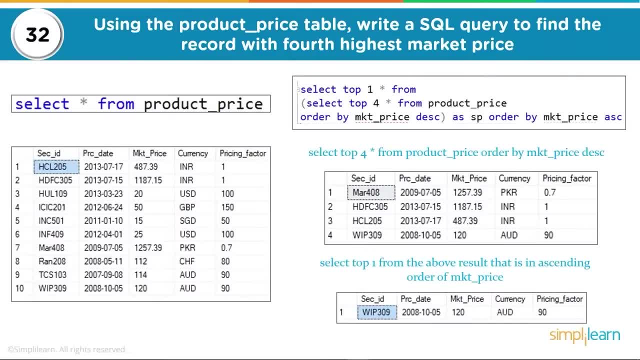 and then we're going to reverse that, and then we're going to reverse that order and do descending order, and do descending order and do descending, and we're going to take the top one of, and we're going to take the top one of, and we're going to take the top one of that which is going to give us the lowest. 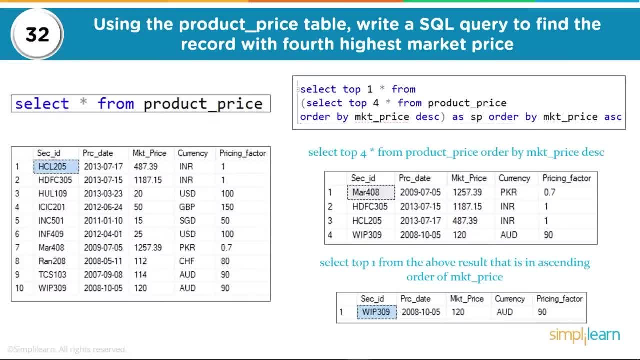 that which is going to give us the lowest, that which is going to give us the lowest value, which would be the fourth greatest value, which would be the fourth greatest value, which would be the fourth greatest one in the list. one in the list, one in the list. from the product price table, find the: 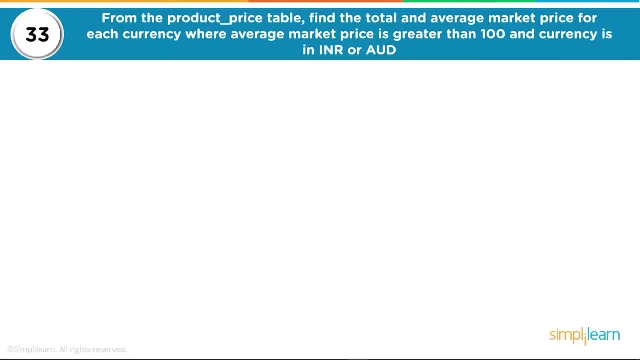 from the product price table. find the. from the product price table. find the total and average market price for each total and average market price for each total and average market price for each currency where the average market price currency. where the average market price currency where the average market price is greater than 100. and currency. 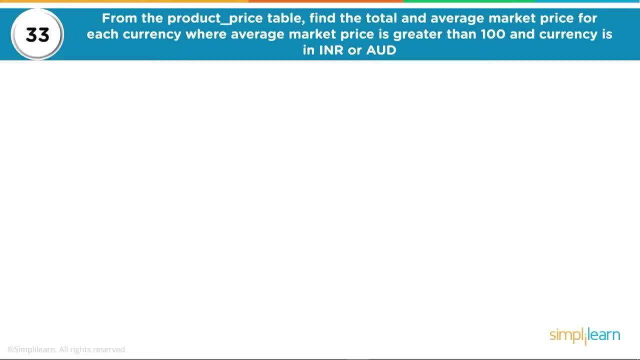 is greater than 100 and currency is greater than 100, and currency is in the inr or the aud is in the inr or the aud is in the inr or the aud. so so so inr or aud india ruple or inr or aud india ruple, or. 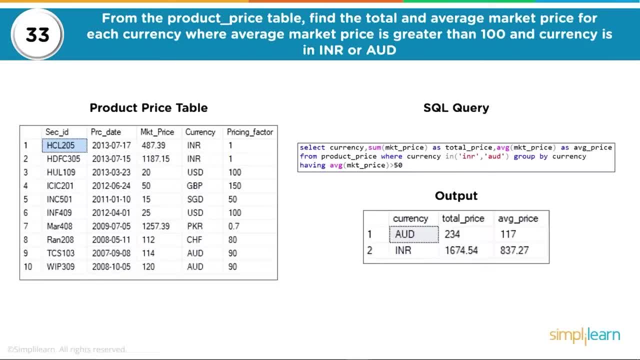 inr or aud, india ruple or australia dollar, australia dollar, australia dollar. you can see over here the sql query. if you can see over here the sql query. if you can see over here the sql query. if you had trouble putting this together, you had trouble putting this together. 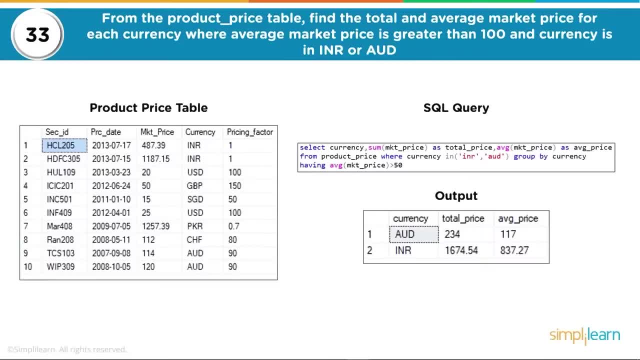 you had trouble putting this together. you might actually do some of it in. you might actually do some of it in. you might actually do some of it in reverse, reverse, reverse. and you can see right here where the and you can see right here where the and you can see right here where the average market price is greater than 50. 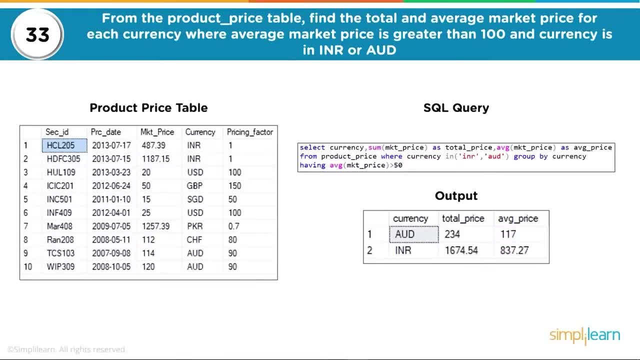 average market price is greater than 50. average market price is greater than 50. remember we use having, not where at the. remember we use having not where at the. remember we use having not where at the end because it's part of the group. so end because it's part of the group. so 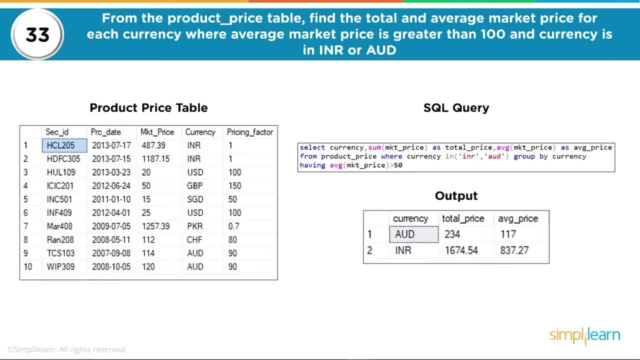 You can see over here the SQL query. If you had trouble putting this together, you might actually do some of it in reverse- And you can see right here where the average market price is greater than 50. Remember we use having not where at the end because it's part of the group. 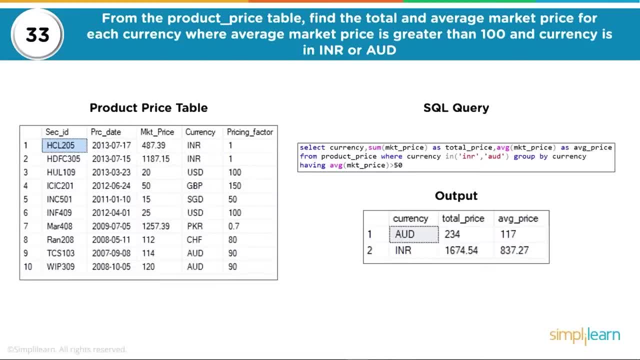 So group by currency, Because we want the total, We want those two currencies And we want the currency India Rupel the INR or the AUD And as you keep going backwards, we're actually going to be selecting the currency, the sum. 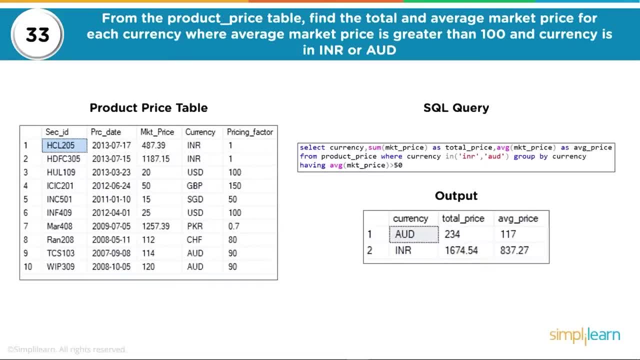 of the market price as total price and the average market price as average price. So there's our select. It's going to come from the product price, which is just our table over there, And then we have where our currency is in. 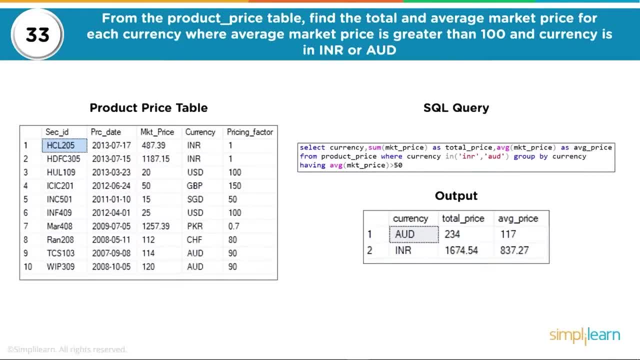 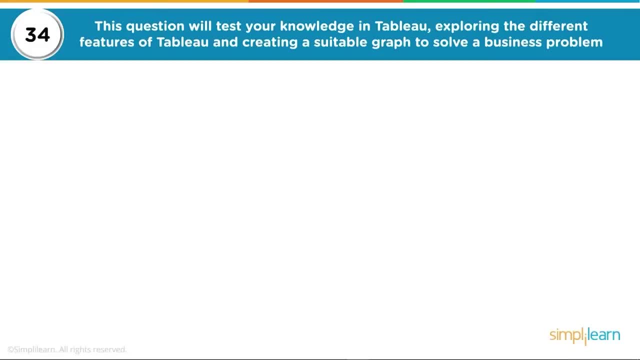 And, like I said, you can put it together however you want, but hopefully you got to the end there. So this question will test your knowledge. It's going to test your knowledge in Tableau, exploring the different features of Tableau and creating a suitable graph to solve a business problem. 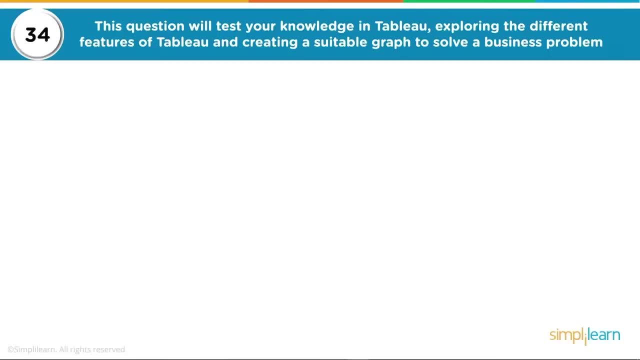 And of course, Tableau is very visual in its use, So it's very hard to test it without actually just getting your hands on. And if you can't visualize some of this and how to do it, then you should go back and refresh yourself. 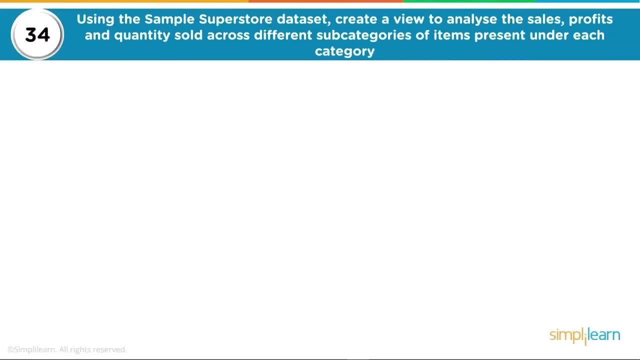 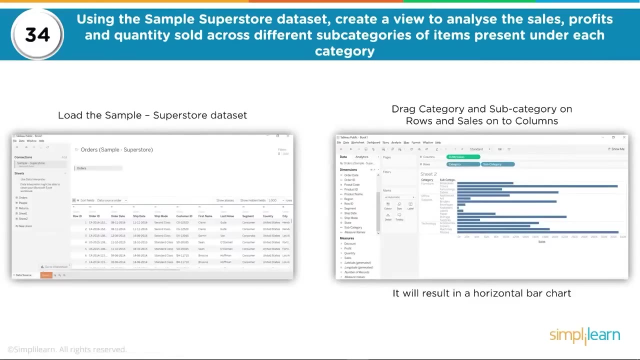 Using the sample superstore data set, create a view to analyze the sales, profits and quantity sold across different subcategories of items. Okay, So the first step is to go ahead and load the sample superstore data set. So make sure you know how to load the sample, the superstore data set that's underneath. 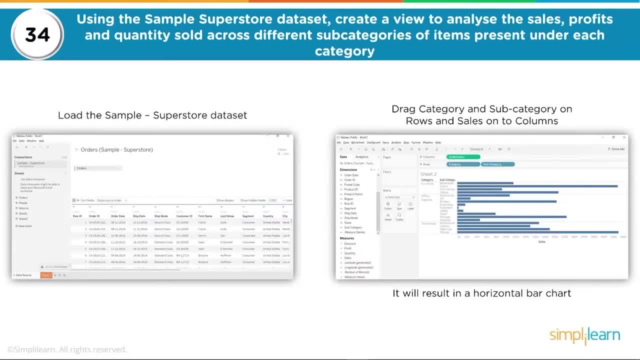 either the connect button in the upper left or the Tableau icon up there and be able to pull in the data set And then, once you've done that, you just drag the category and subcategory on rows and salaries onto columns. It will result in a horizontal bar chart. 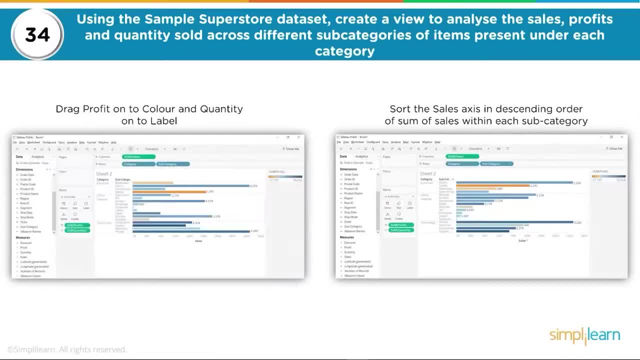 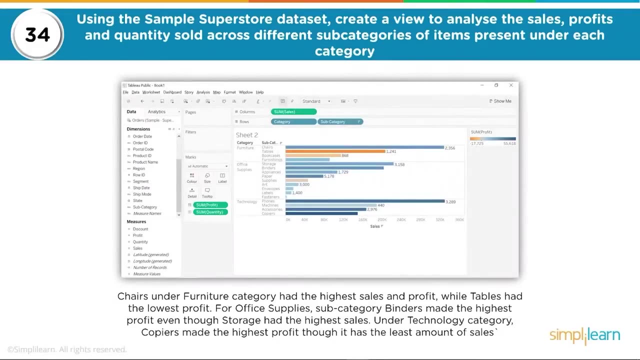 So in this one we're just going to drag profit onto color and quantity onto label. Sort the sales axes in descending order of sum and sales within each subcategory And if you're at home doing this, you'll see that chairs under furniture category had the 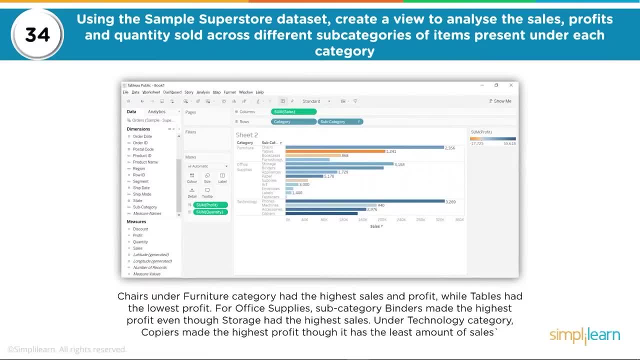 highest sales and profit, while tables had the lowest profit. For office supplies, subcategory binders made the highest profit, even though storage had the highest sales. Under technology category binders made the highest profit. Under category, copiers made the highest profit, though it was the least amount of. 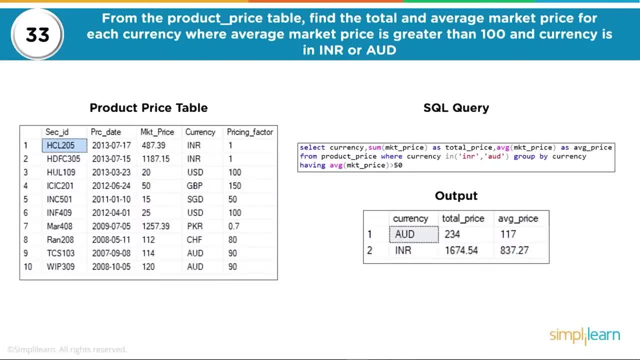 end because it's part of the group. so, group by currency, because we want those, group by currency, because we want those, group by currency, because we want those two currencies and we want the currency- two currencies, and we want the currency- two currencies, and we want the currency- india rupe, the inr or the aud. 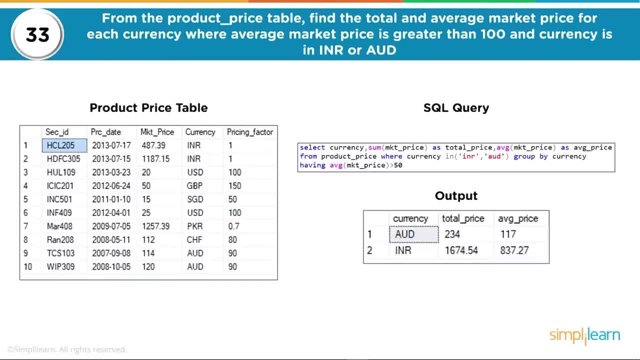 india rupe the inr or the aud, india rupe the inr or the aud. and as you keep going backwards, we're, and, as you keep going backwards, we're, and as you keep going backwards, we're actually going to be selecting the, actually going to be selecting the. 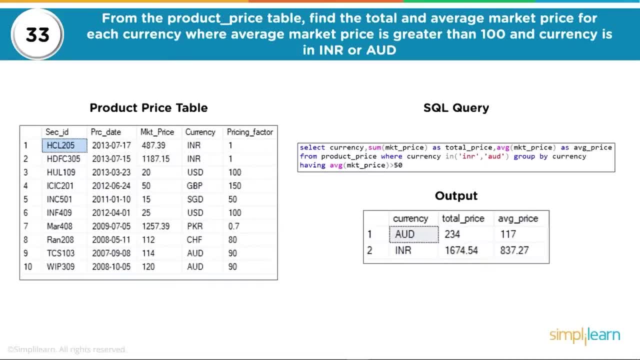 actually going to be selecting the currency: the sum of the market price as currency, the sum of the market price as currency, the sum of the market price as total price and the average marketplace total price and the average marketplace total price and the average marketplace as average price. so there's our select. 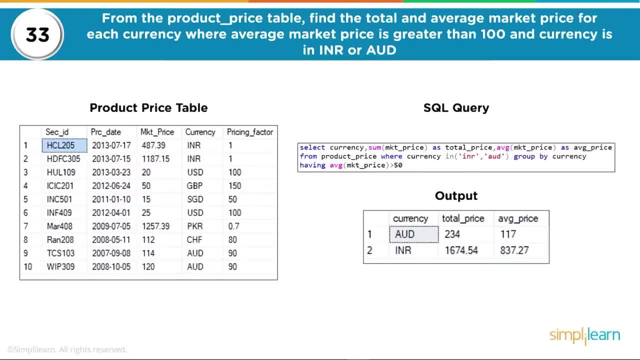 as average price. so there's our select as average price. so there's our select. it's going to come from the product. it's going to come from the product. it's going to come from the product. price which is just our table over there. price which is just our table over there. 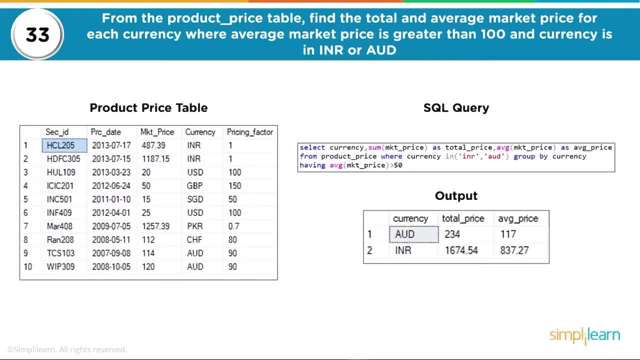 price, which is just our table over there, and then we have where our currency is, and then we have where our currency is, and then we have where our currency is in uh, and, like i said, you can put it in. uh, and, like i said, you can put it. 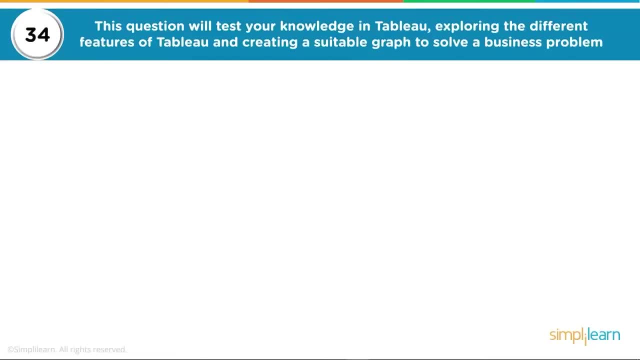 in uh, and, like i said, you can put it together however you want, but hopefully together however you want, but hopefully together however you want, but hopefully you got to the end there. you got to the end there, you got to the end there. so this question will test your. 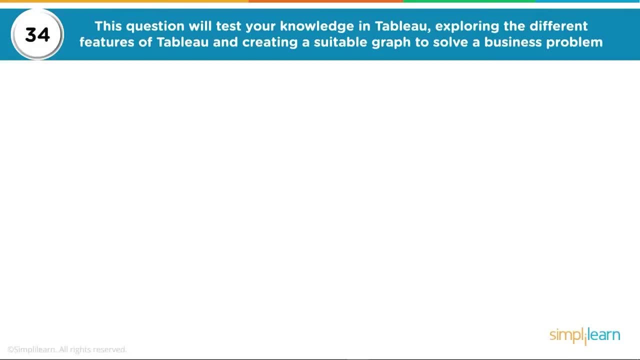 so this question will test your. so this question will test your knowledge in tablou. exploring the knowledge in tablou, exploring the knowledge in tablou, exploring the different features of tablou and different features of tablou and different features of tablou and creating a suitable graph to solve a. 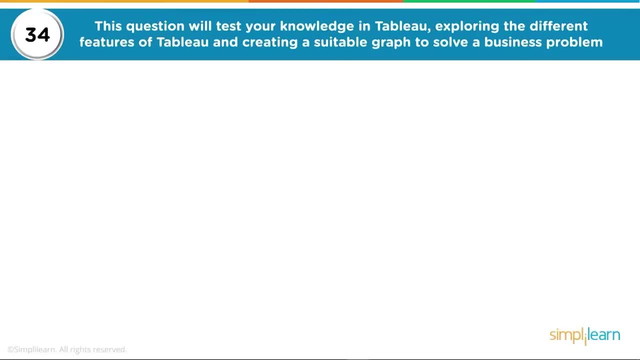 creating a suitable graph to solve a. creating a suitable graph to solve a business problem, business problem, business problem. and of course, tablou is very visual in, and of course tablou is very visual in, and of course, tablou is very visual in its use, so it's very hard to test it. 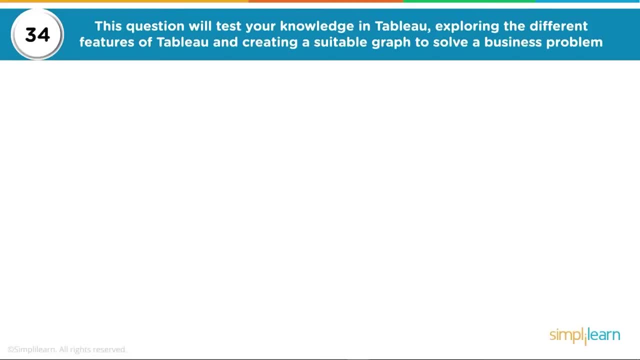 its use, so it's very hard to test it, its use, so it's very hard to test it without actually just getting your hands, without actually just getting your hands, without actually just getting your hands on, and if you can't visualize some of on and if you can't visualize some of 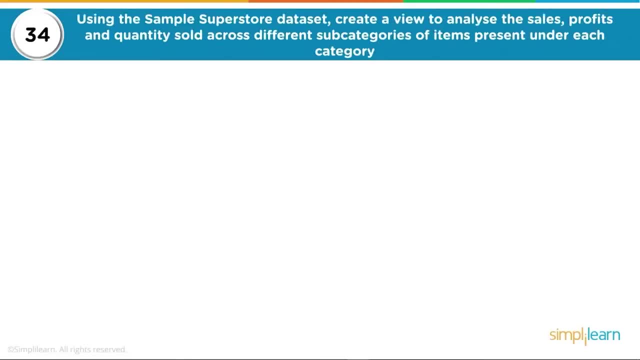 on, and if you can't visualize some of this and how to do it, then you should go this and how to do it, then you should go this and how to do it. then you should go back and refresh yourself back and refresh yourself back and refresh yourself using the sample superstore data set. 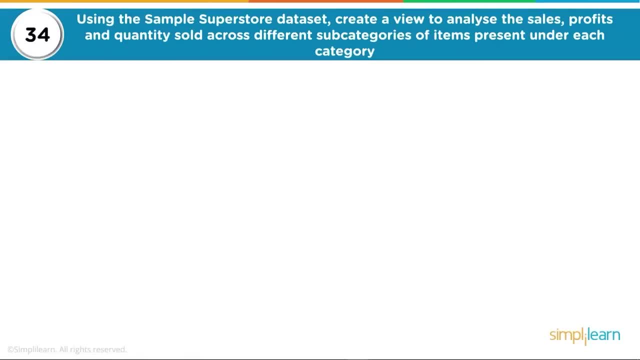 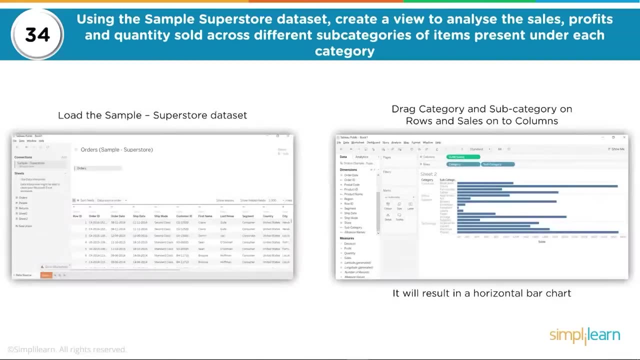 using the sample superstore data set. using the sample superstore data set, create a view to analyze the cells. create a view to analyze the cells. create a view to analyze the cells. so make sure you know how to load the. so make sure you know how to load the. 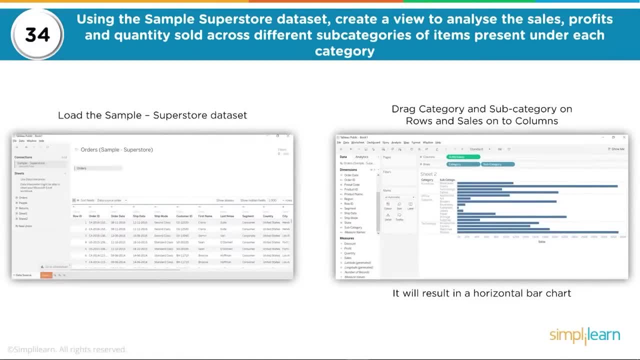 so make sure you know how to load the sample: the superstore data set. that's sample, the superstore data set. that's sample. the superstore data set. that's underneath: either the connect button in underneath, either the connect button in underneath, either the connect button in the upper left. 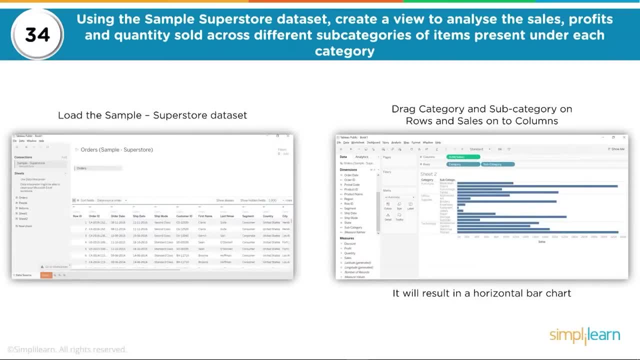 the upper left. the upper left or the tablou icon up there and be able. or the tablou icon up there and be able. or the tablou icon up there and be able to pull in the data set. to pull in the data set. 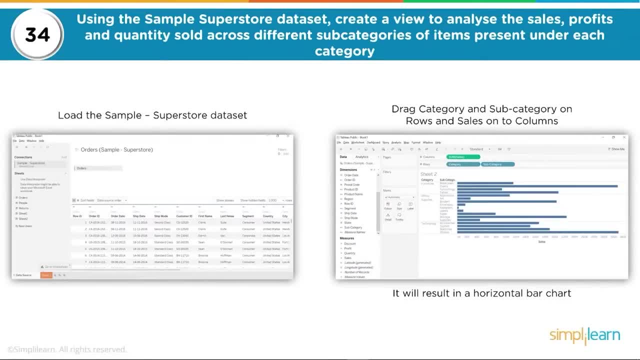 to pull in the data set and then, once you've done that, you just. and then, once you've done that, you just. and then, once you've done that, you just drag the category and subcategory on. drag the category and subcategory on. drag the category and subcategory on rows and salaries onto columns. it will. 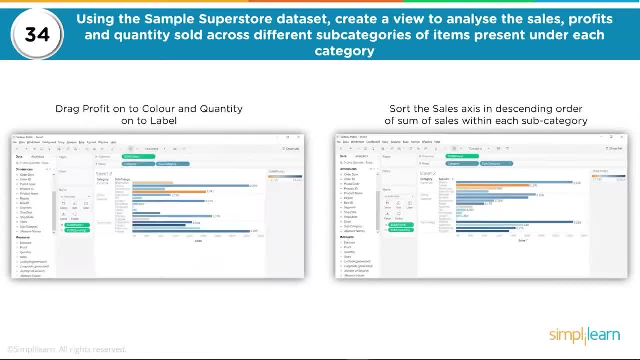 rows and salaries onto columns. it will rows and salaries onto columns. it will result in a horizontal bar chart. result in a horizontal bar chart. result in a horizontal bar chart. so in this one, we're just going to drag. so in this one, we're just going to drag. 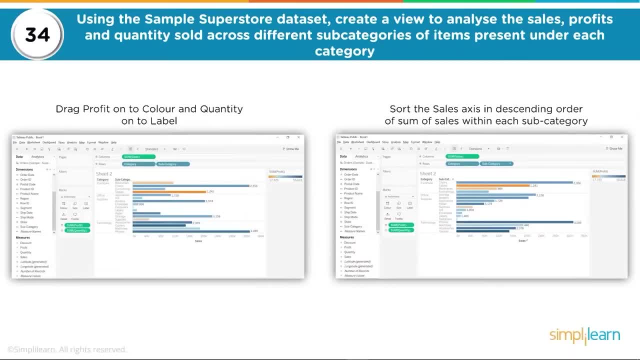 so in this one we're just going to drag profit onto color and quantity onto profit onto color and quantity onto profit onto color and quantity onto label. sort the sales axes in descending label. sort the sales axes in descending label. sort the sales axes in descending order of sum and cells within each. 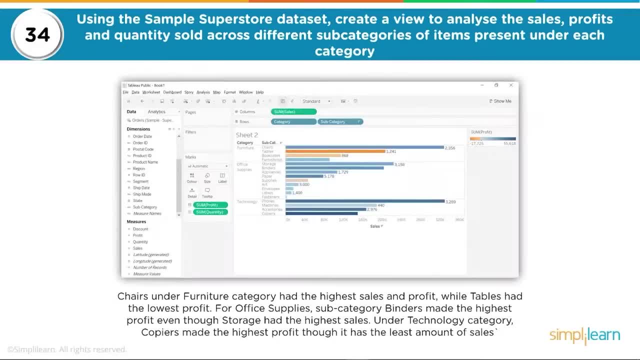 order of sum and cells within each order of sum and cells within each subcategory, subcategory, subcategory. and. if you're at home doing this, you'll, and if you're at home doing this, you'll. and if you're at home doing this, you'll see that chairs under furniture. 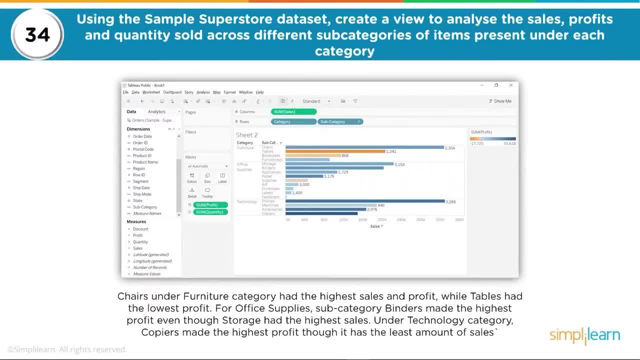 see that chairs under furniture. see that chairs under furniture. binders made the highest profit. even binders made the highest profit. even binders made the highest profit, even though storage had the highest cells. though storage had the highest cells, though storage had the highest cells. under technology category, copiers made. 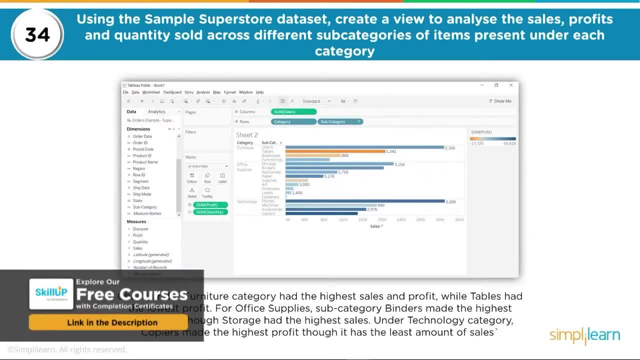 under technology category copiers made under technology category copiers made the highest profit, the highest profit, the highest profit, though it was the least amount of cells, though it was the least amount of cells, though it was the least amount of cells. let's work to create a dual axes chart. 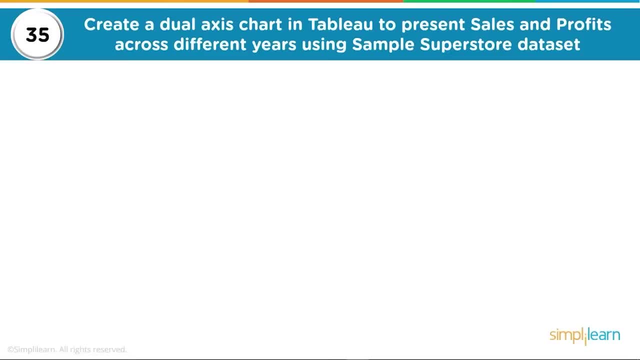 let's work to create a dual axes chart. let's work to create a dual axes chart in tableau. to present cells and profits in tableau. to present cells and profits in tableau. to present cells and profits across different years. using sample across different years. using sample across different years. using sample superstore dataset. 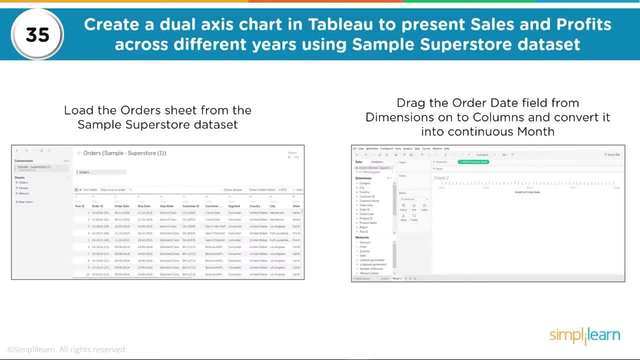 superstore dataset. superstore dataset. load the orders sheet from the sample. load the orders sheet from the sample. load the orders sheet from the sample. superstore dataset. superstore dataset. superstore dataset. drag the order data field from the. drag the order data field from the. drag the order data field from the dimensions onto columns and convert it. 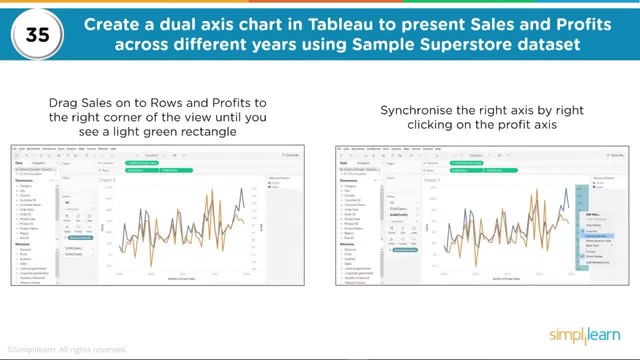 dimensions onto columns and convert it dimensions onto columns and convert it into continuous month, into continuous month, into continuous month. drag cells onto rows and profits to the drag cells onto rows and profits to the drag cells onto rows and profits to the right corner of the view, until you see a. 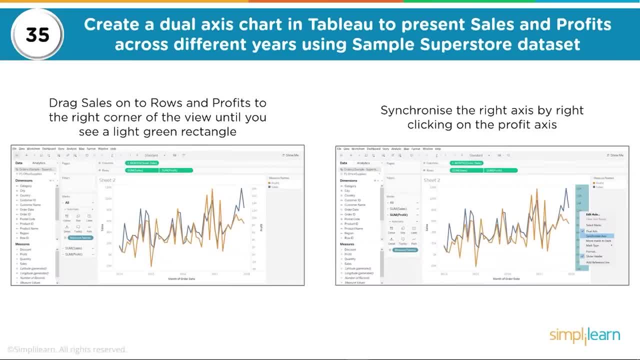 right corner of the view, until you see a right corner of the view, until you see a light green light, green light, green rectangle one of those things. if you rectangle one of those things, if you rectangle one of those things, if you haven't done this hands-on, you don't. 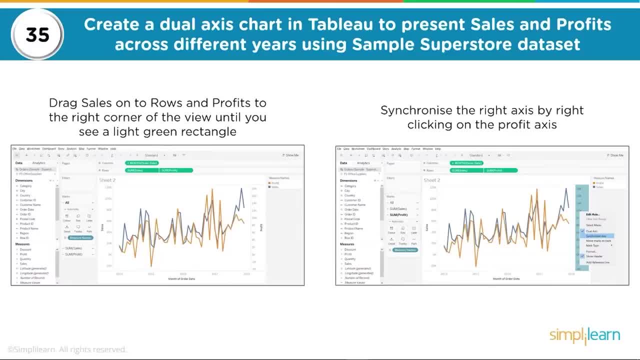 haven't done this hands-on. you don't haven't done this hands-on. you don't know what you're doing. your run into a know what you're doing. your run into a know what you're doing. your run into a buying signal: be just kind of dropping. 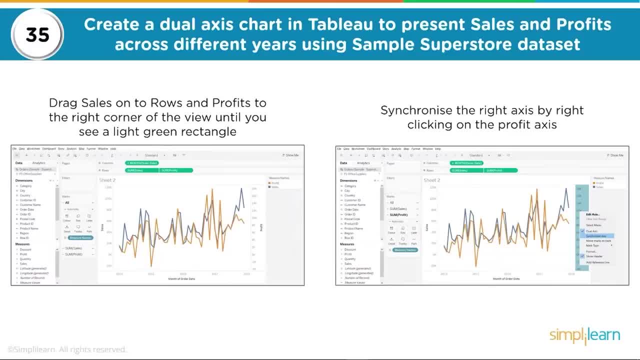 buying signal. be just kind of dropping buying signal. be just kind of dropping it and wondering what happened it and wondering what happened it and wondering what happened. synchronize the right axes by. synchronize the right axes by. synchronize the right axes by right-clicking on the profit axes and. 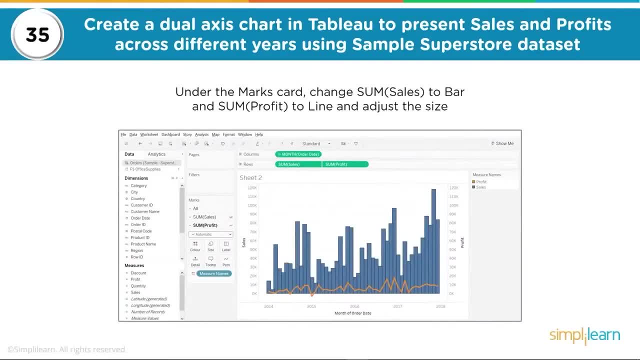 right-clicking on the profit axes and right-clicking on the profit axes, and then let's finalize it by going under. then let's finalize it by going under. then let's finalize it by going under. the marks card: change some cells to bar. the marks card: change some cells to bar. 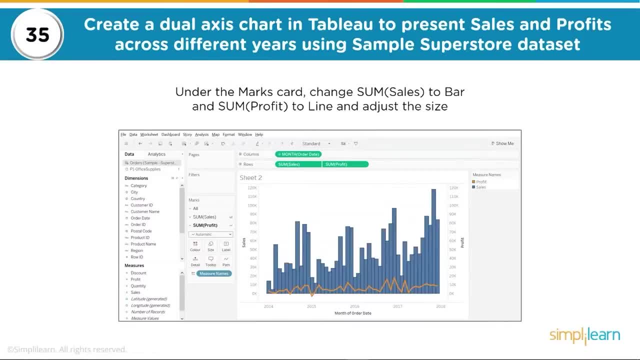 the marks card, change some cells to bar and some profit to line and adjust the and some profit to line and adjust the and some profit to line and adjust the size, and then we have a nice display size. and then we have a nice display size and then we have a nice display that we can either print out or save, and 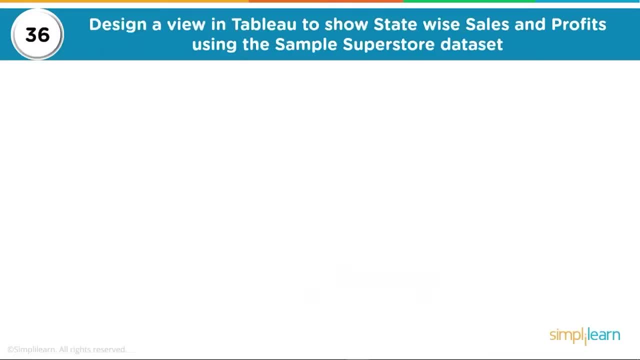 that we can either print out or save, and that we can either print out or save and send off to the shareholders. let's go send off to the shareholders. let's go send off to the shareholders. let's go ahead and do one more tablou design a. 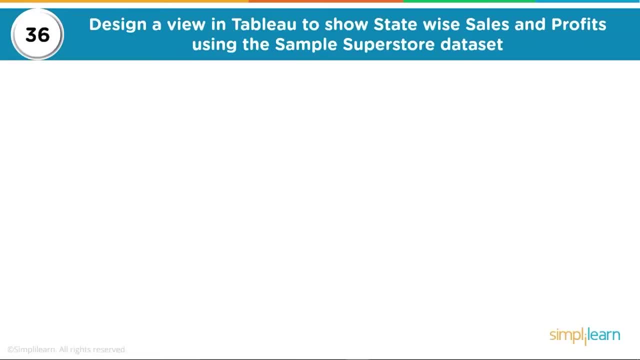 ahead and do one more tablou design a ahead and do one more tablou design a view and tablou to show state wise cells- view and tablou to show state wise cells- view and tablou to show state wise cells and profits using the sample superstore. 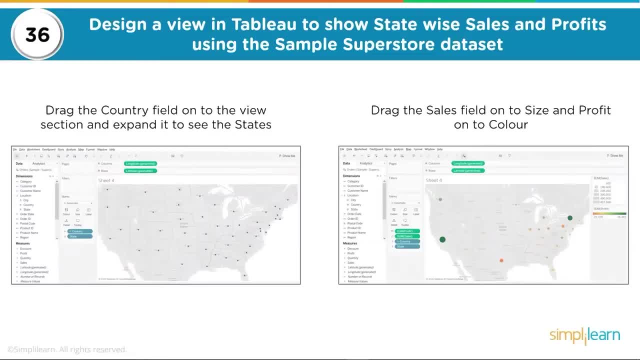 and profits using the sample superstore and profits using the sample superstore. data set in. here you go ahead and drag data set in here you go ahead and drag data set in. here you go ahead and drag the country filled on to the view section. the country filled on to the view section. 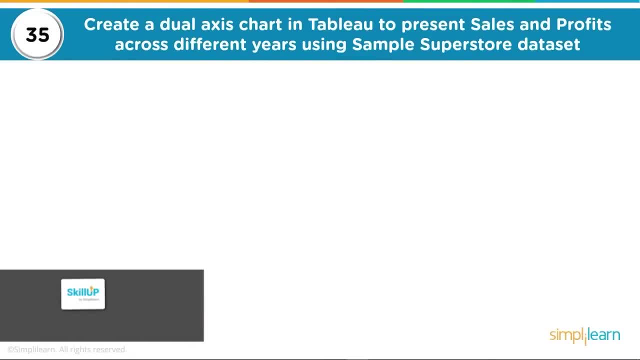 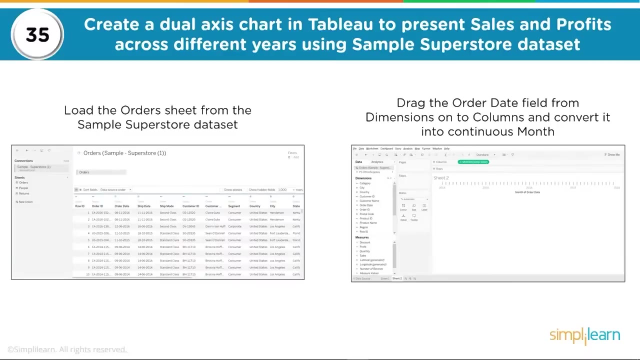 sales. Let's work to create a dual axes chart in Tableau to present sales and profits across different years using sample superstore data set. Load the orders sheet from the sample superstore data set. Drag the order data field from the dimensions onto columns and convert it into continuous. 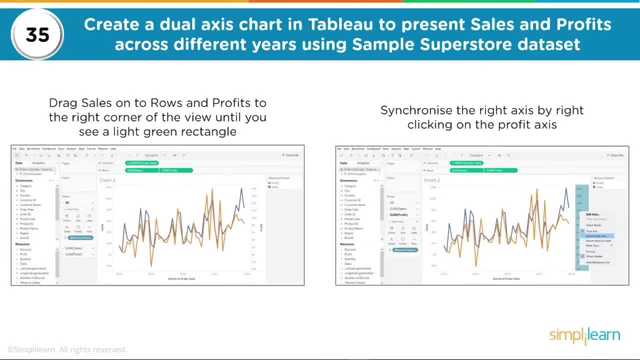 month. Drag cells onto rows and profits to the right corner of the view until you see a light green rectangle, One of those things. if you haven't done this hands-on and you don't know what you're doing, you're going to run into a bind because you're going to be just kind of dropping it and wondering. 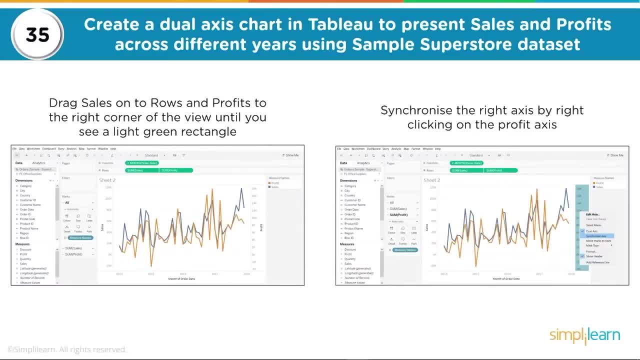 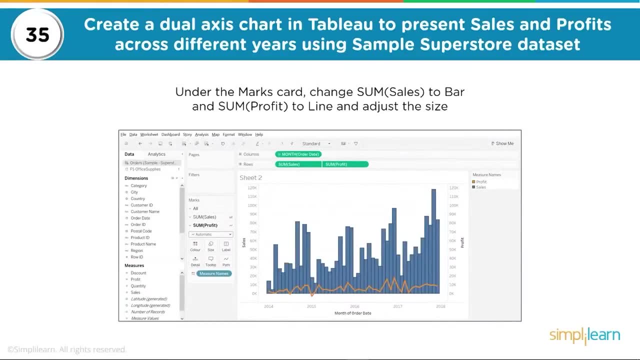 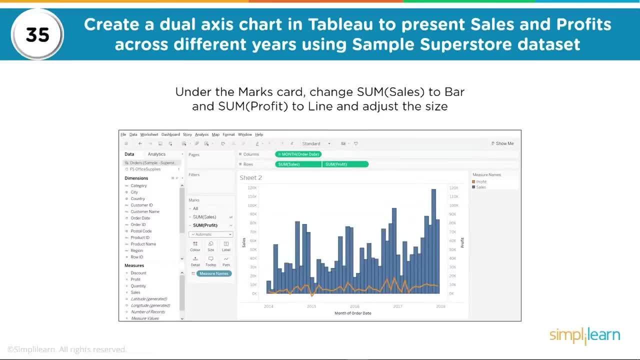 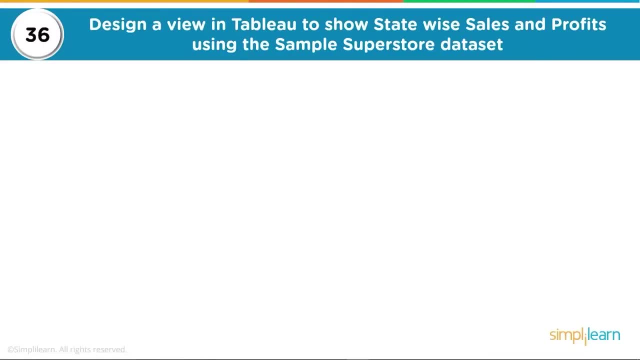 nice, And then we have a nice display that we can either print out or save and send off to the shareholders. Let's go ahead and do one more at Tableau Design: a view in Tableau to show state-wise sales and profits using the sample superstore. 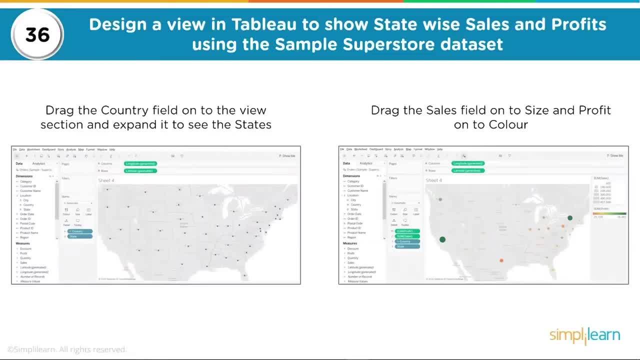 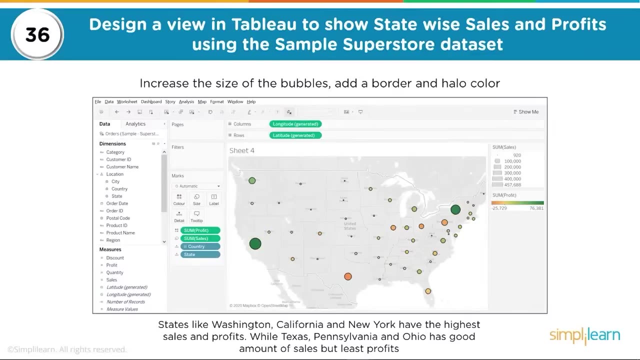 data set In here. you go ahead and drag the country field onto the view section and expand it to see the states. Drag the states field onto size and profit onto color. Increase the value. Increase the value. Increase the size of the bubbles. add a border and a halo color. 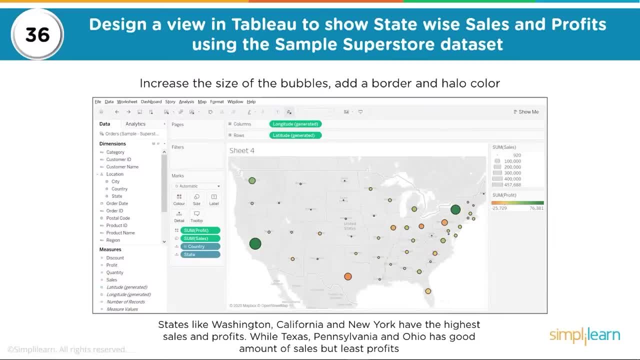 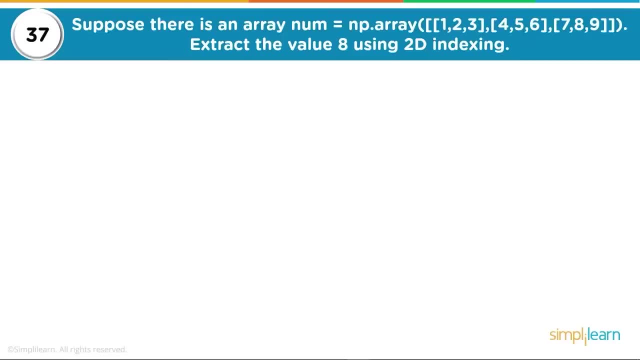 States like Washington, California and New York have the highest sales and profits, while Texas, Pennsylvania and Ohio have a good amount of sales but the least amount of profits. We'll go ahead and skip back to Python numpy. Suppose there is an array number equals np or numpy- if you're using numpy, depending. 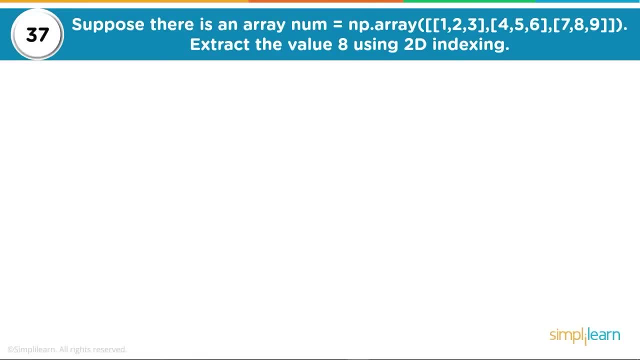 on how you set that up array and we just have 1 to 9 broken up into three groups. Extract the value 8 using 2D indexing So you can see on the left we have our import numpy as np number equals our np array. If we print the number, we have 1,, 2,, 3,, 4,, 5,, 6,, 7,, 8, 9.. Since the value 8 is present in the second row and first column, we use the same index. 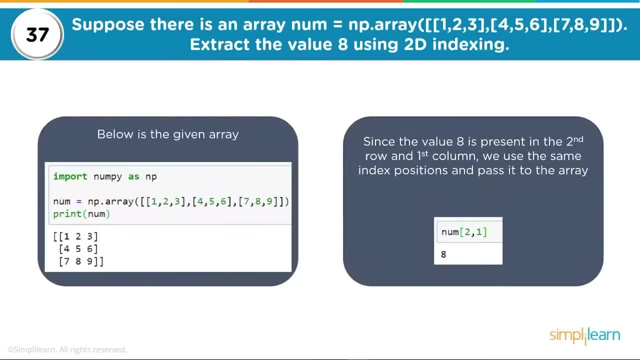 position and pass it to the array And you just have number 2,, 1, and you get 8.. And remember, we're in Python, so you start at 0,, not 1, like you do in Excel. So let's go ahead and do that. 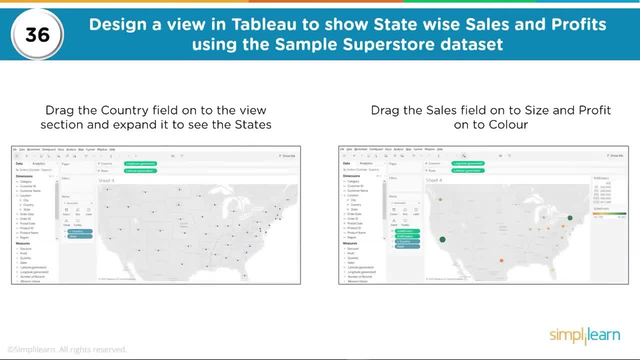 the country filled on to the view section and expand it. to see the states drag the and expand it. to see the states drag the and expand it. to see the states drag the state's filled on to size and profit on. state's filled on to size and profit on. 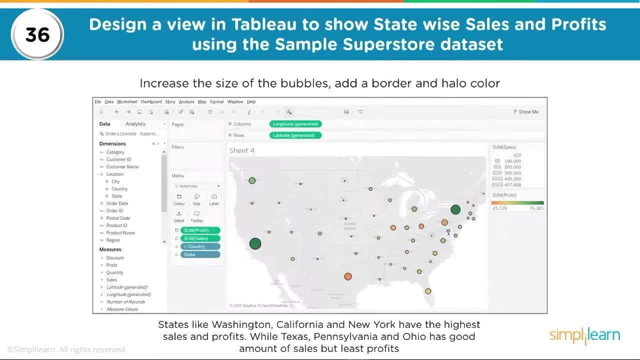 state's filled on to size and profit on to color. increase the size of the bubbles to color. increase the size of the bubbles to color. increase the size of the bubbles at a border and a halo color states like: at a border and a halo color states like: 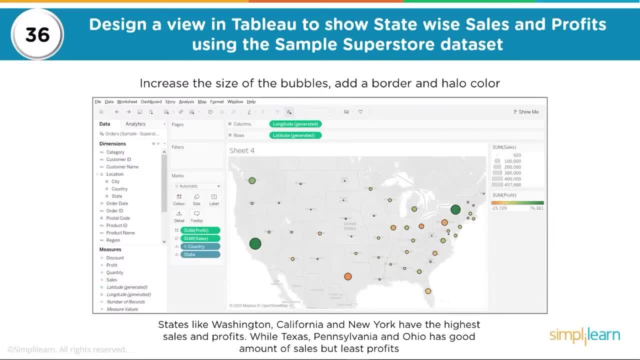 at a border and a halo. color states like Washington, California, New York have the Washington California, New York have the Washington California, New York have the highest sales and profits, while Texas highest sales and profits, while Texas highest sales and profits, while Texas, Pennsylvania and Ohio have a good amount. 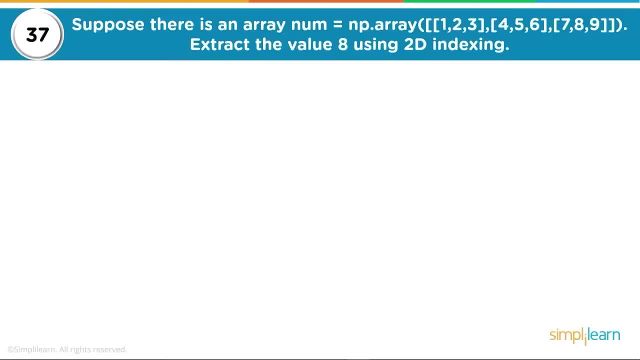 Pennsylvania and Ohio have a good amount. Pennsylvania and Ohio have a good amount of sales, but the least amount of of sales, but the least amount of of sales, but the least amount of profits, profits, profits. we'll go ahead and skip back to Python. we'll go ahead and skip back to Python. 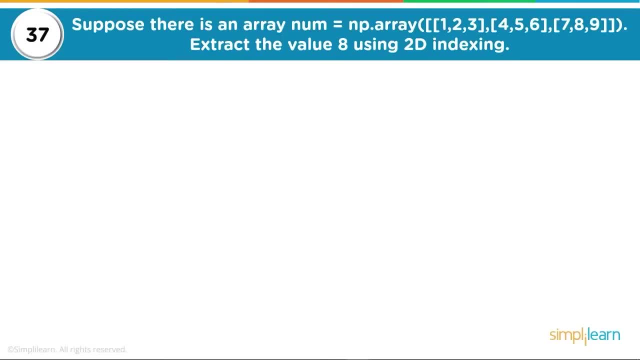 we'll go ahead and skip back to Python. numpy. suppose there is an array number. numpy. suppose there is an array number. numpy. suppose there is an array number equals NP or numpy. if you're using numpy, equals NP or numpy if you're using numpy, equals NP or numpy if you're using numpy, depending why you set it up. dot array. 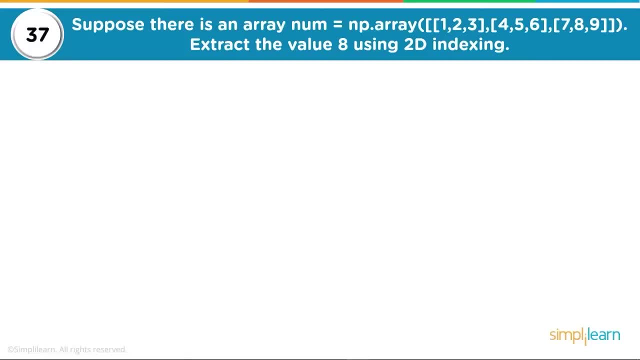 depending why you set it up dot array, depending why you set it up dot array and we just have one to nine broken up, and we just have one to nine broken up, and we just have one to nine broken up into three groups. extract the value 8. 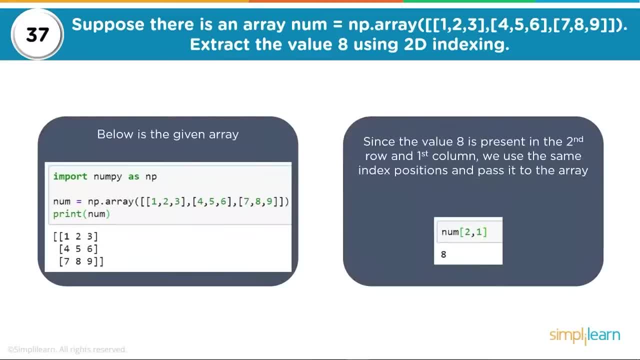 into three groups. extract the value 8 into three groups. extract the value 8 using 2d indexing so you can see on the using 2d indexing. so you can see on the using 2d indexing. so you can see on the left we have our import numpy as NP. 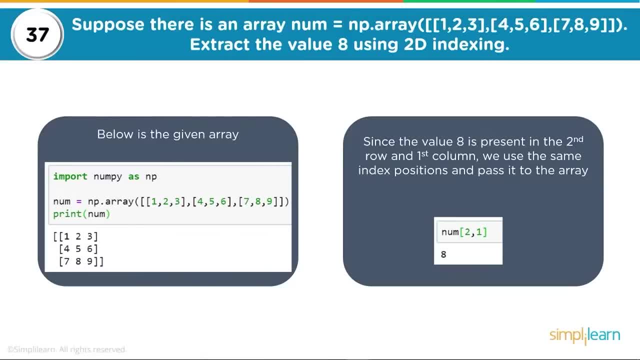 left we have our import numpy as NP. left we have our import numpy as NP. number equals our NP array. if we print number equals our NP array. if we print number equals our NP array. if we print the number, we have 1, 2, 3, 4, 5, 6, 7, 8, 9. the number we have: 1, 2, 3, 4, 5, 6, 7, 8, 9. the number we have: 1, 2, 3, 4, 5, 6, 7, 8, 9, since the value 8 is present in the 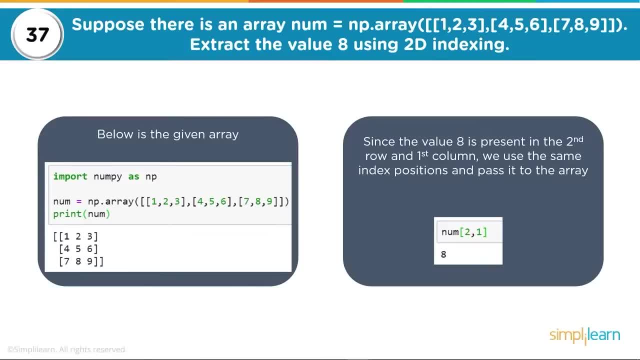 since the value 8 is present in the, since the value 8 is present in the second row and first column, we use the second row and first column. we use the second row and first column. we use the same index position and pass it to the same index position and pass it to the. 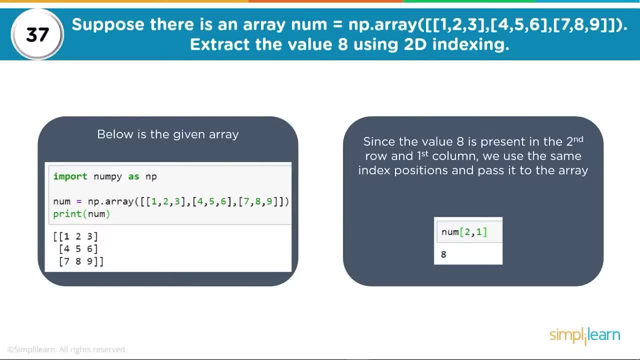 same index position and pass it to the working between Excel and Python, where I working between Excel and Python, where I working between Excel and Python, where I just kind of flip, and usually it's the just kind of flip, and usually it's the just kind of flip and usually it's the Excel that messes up because I do a lot. 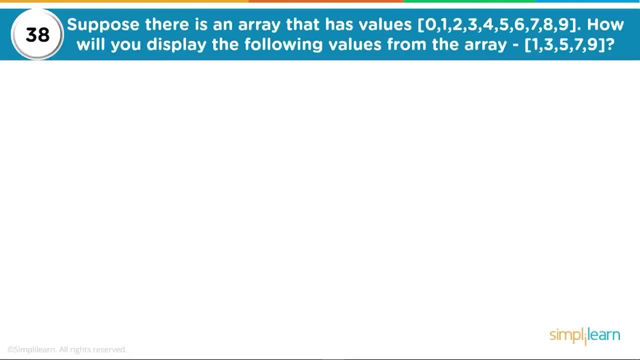 Excel that messes up because I do a lot. Excel that messes up because I do a lot more programming. suppose there is an more programming. suppose there is an more programming. suppose there is an array that has value 0- 1 all the way up. array that has value 0- 1 all the way up. 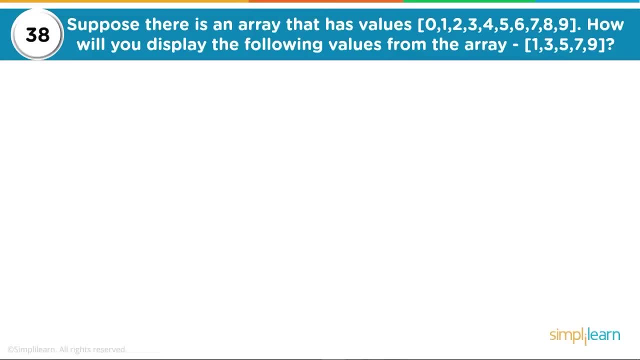 array that has value 0, 1, all the way up to 9. how will you display the following to 9? how will you display the following to 9: how will you display the following values from the array: 1, 3, 5, 7, 9, so. 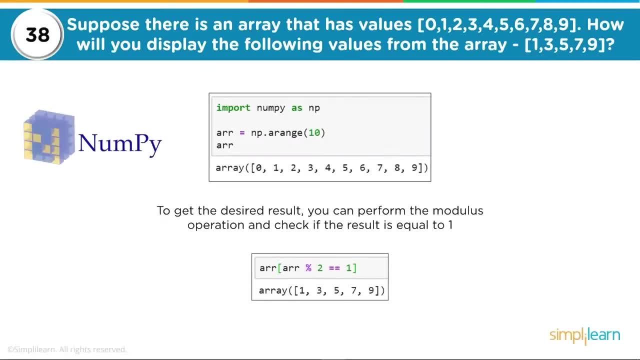 values from the array 1, 3, 5, 7, 9. so values from the array 1, 3, 5, 7, 9. so first of all, we go ahead and create the first of all, we go ahead and create the first of all. we go ahead and create the array in P dot, a range of 10 which goes. We'll go ahead and import numpy as np number equals our np array. If we print the number, we have 1, 2,, 3,, 4,, 5,, 6,, 7,, 8, 9.. 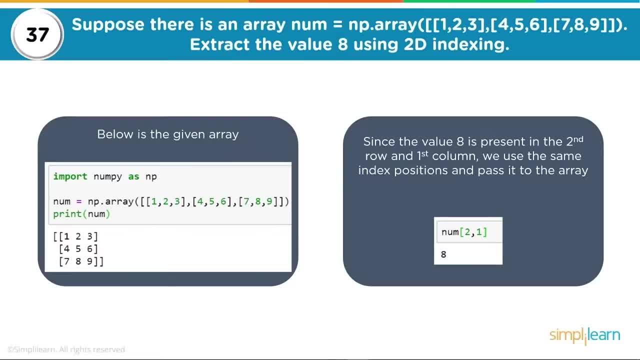 Since the value 8 is present in the second row and first column, we use the same index position and pass it to the array And you just have number 2,, 1, and you get 8.. Since the value 8 is present in the second row and first column, we use the same index. 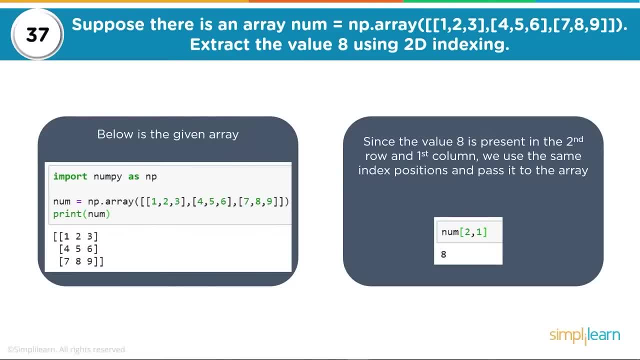 position and pass it to the array And you just have number 2, 1, and you get 8.. And remember, we're in Python, so you start at 0,, not 1 like you do in Excel. And remember, we're in Python, so you start at 0,, not 1 like you do in Excel. It always gets me if I'm working between Excel and Python where I just kind of flip, and usually it's the Excel that messes up, because I do a lot more programming. So let's go ahead and import numpy as np. number equals our np array. 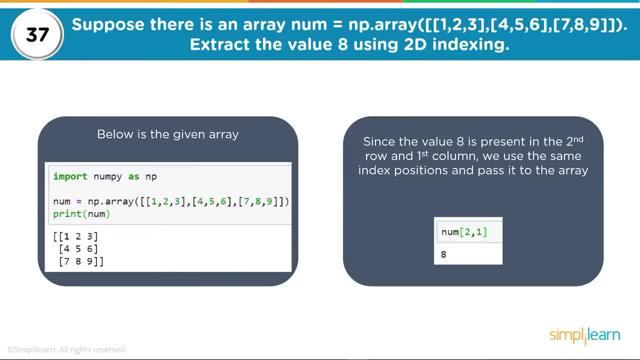 If we print the number, we have 1,, 2,, 3,, 4,, 5,, 6,, 7,, 8, 9.. 3,, 3,, 5,, 6,, 7,, 9.. 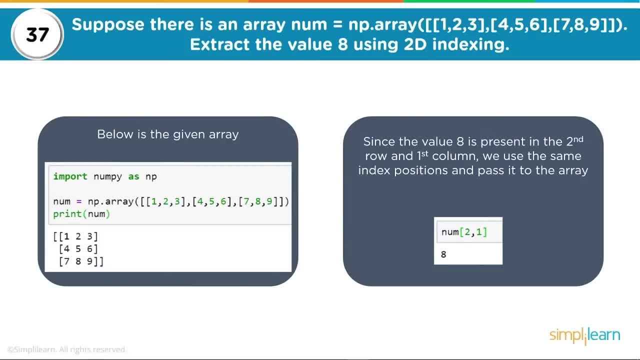 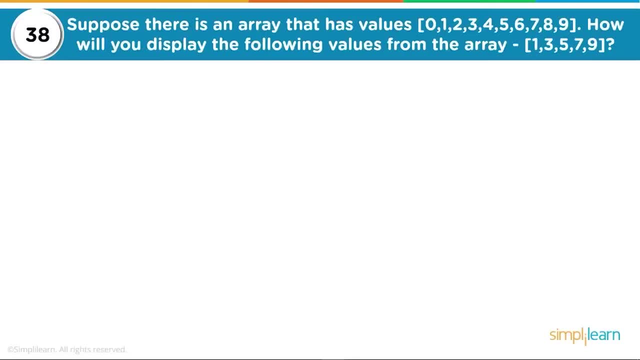 And then this is actually the number 2, 1, and it's present in the second row, and usually you just have number 2, 2, 5,, 6,, 7, 8.. That's a pretty nice array. 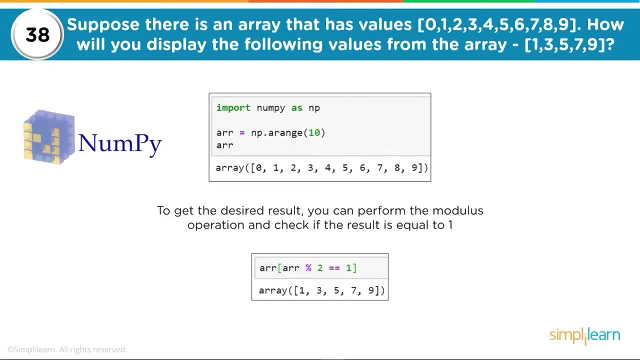 All right. So, first of all, we go ahead and create the array nparange, which goes from 0 to 9, because there's 10 numbers in it, but we don't include the 10. We print it out. The first thing you want to do is what's going on here with 1,, 3,, 5,, 7,, 9?? 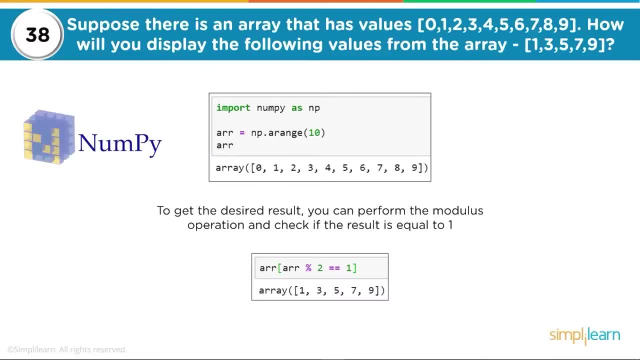 Well, if we divide by 2, there's going to be a remainder equal to 1.. And then, from Python, remember that if you use the percentage sign, you get the remainder on there. So the remainder is 1, and then you have your numpy array. 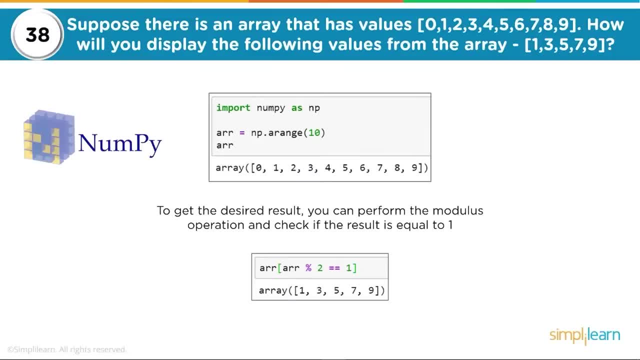 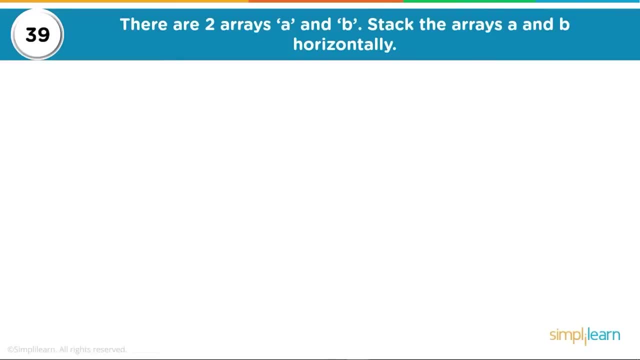 And then we just want to do a logical statement of all values that have a remainder of 1, and that generates our nice 1, 3,, 5,, 7, 9.. There are two arrays, A and B. Stack the arrays A and B horizontally. 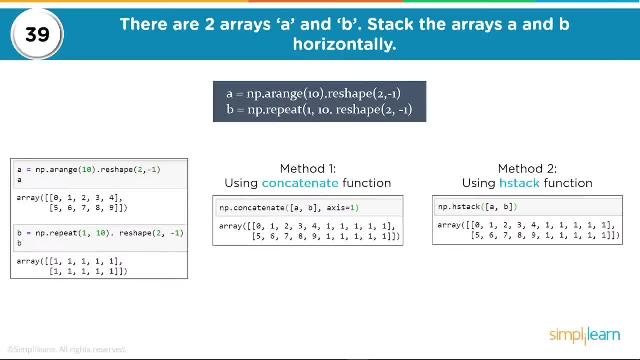 Boy, these horizontal vertical questions will get you every time, And in numpy we go ahead and we've created two different arrays over here: A and B. The first one is your concatenate npconcatenate A and B on axes equal 1.. 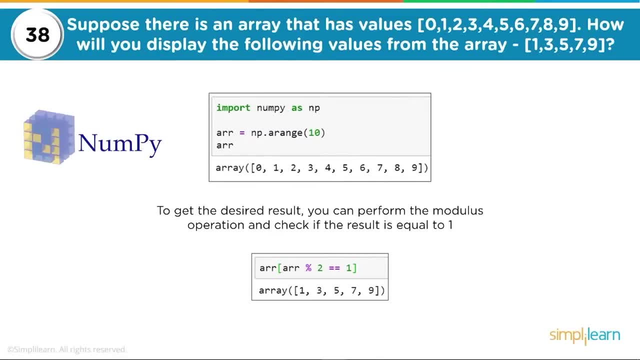 array in P dot a range of 10 which goes. array in P dot a range of 10 which goes from 0 to 9, because there's 10 numbers from 0 to 9, because there's 10 numbers from 0 to 9, because there's 10 numbers in it, but we don't include the 10. we 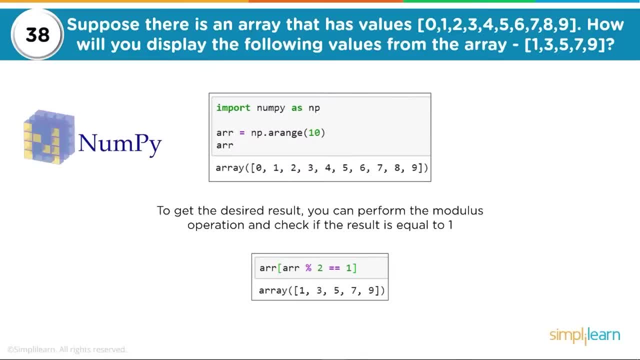 in it, but we don't include the 10. we in it, but we don't include the 10. we print it out. the first thing you want to print it out, the first thing you want to print it out. the first thing you want to do is what's going on here with 1, 3, 5, 7. 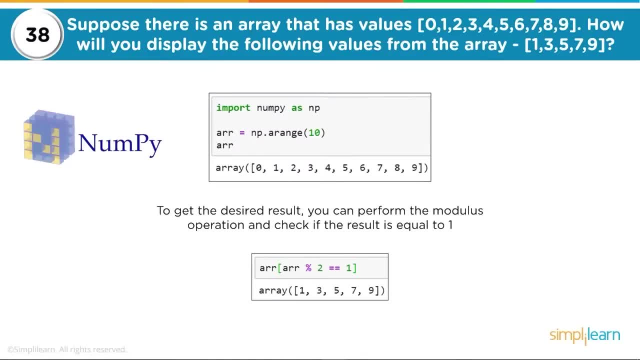 do is what's going on here with 1, 3, 5, 7. do is what's going on here with 1, 3, 5, 7, 9. well, if we divide by 2, there's going 9. well, if we divide by 2, there's going. 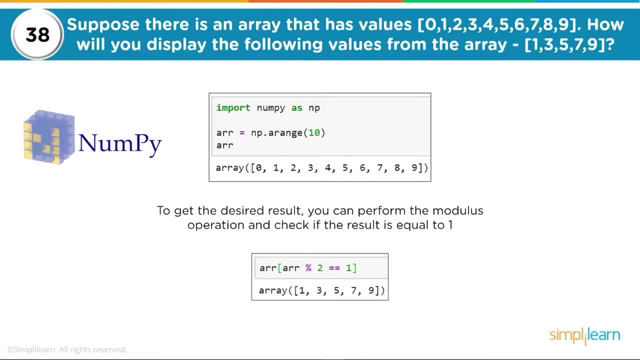 9. well, if we divide by 2, there's going to be a remainder equal to 1, and then to be a remainder equal to 1, and then to be a remainder equal to 1, and then from Python. remember that if you use the from Python, remember that if you use the. 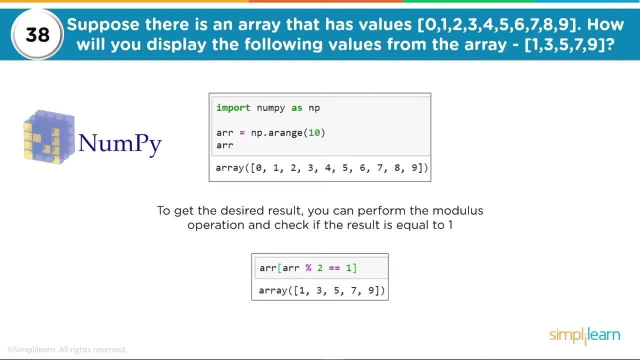 from Python. remember that if you use the percentage sign, you get the remainder on percentage sign. you get the remainder on percentage sign, you get the remainder on there, so the remainder is 1, and then you there, so the remainder is 1, and then you there, so the remainder is 1, and then you have the, your numpy array, and then we. 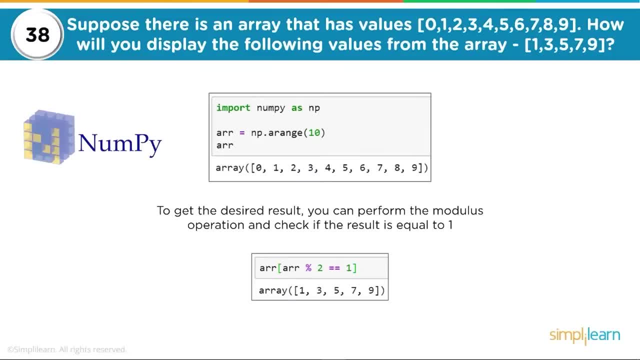 have the your numpy array, and then we have the your numpy array, and then we just want to do a logical statement of just want to do a logical statement, of just want to do a logical statement of all values that have a remainder of 1, all values that have a remainder of 1. 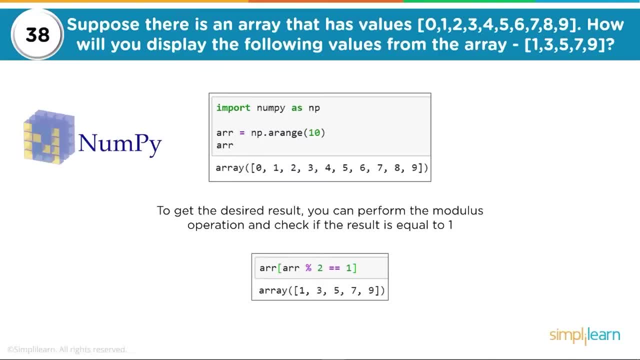 all values that have a remainder of 1 and then generates our nice 1, 3, 5, 7, 9 and then generates our nice 1, 3, 5, 7, 9 and then generates our nice 1, 3, 5, 7, 9. there are two arrays, a and B. stack the. 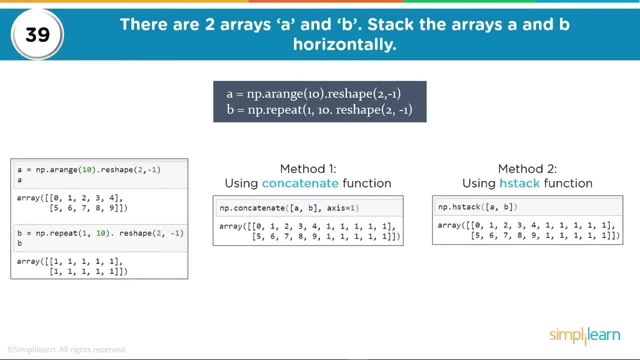 there are two arrays, a and B. stack the. there are two arrays a and B. stack the arrays a and B horizontally boy these arrays a and B horizontally boy these arrays a and B horizontally boy these horizontal vertical questions will get horizontal vertical questions. will get horizontal vertical questions. will get you every time and in numpy we go ahead. 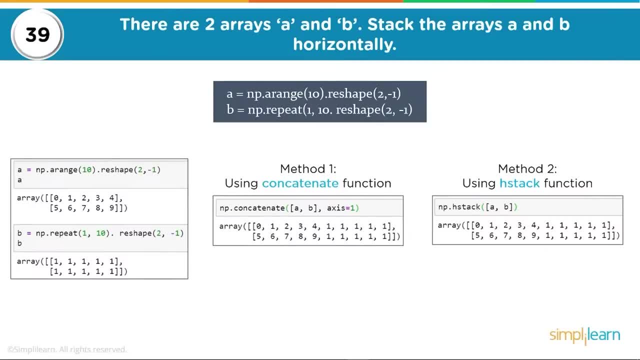 you every time, and in numpy we go ahead, you every time, and in numpy we go ahead. and we've created two different arrays and we've created two different arrays and we've created two different arrays over here, a and B. the first one is your. over here, a and B. the first one is your. 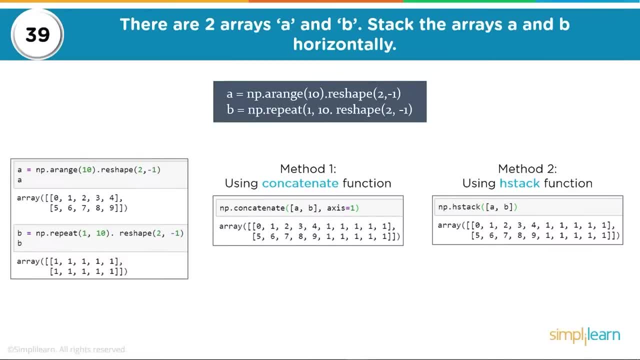 over here: a and B. the first one is your concatenate NP. concatenate a and B. on concatenate NP. concatenate a and B on concatenate NP. concatenate a and B on axes equal 1: that is the same as H stack. axes equal 1, that is the same as H stack. 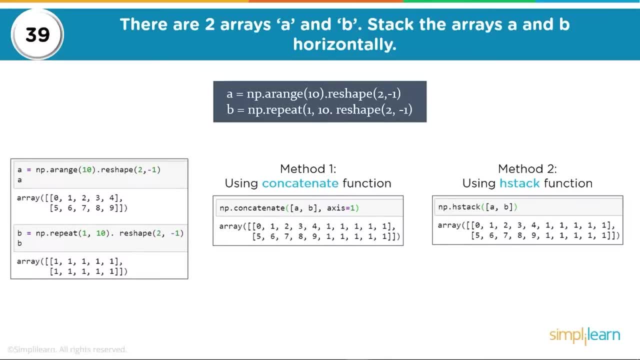 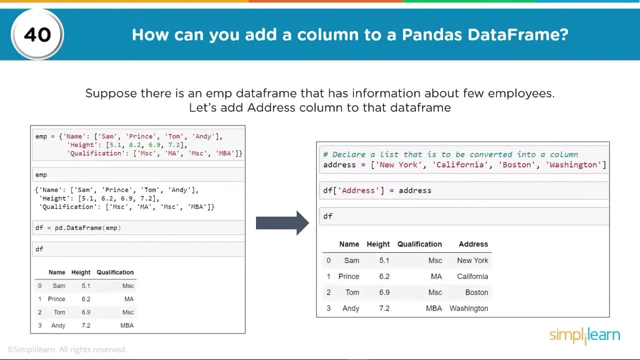 That is the same as HStack And in the back end they're still identical. They run the same, That's all. HStack is a concatenate on axes equals 1.. How can you add a column to a pandas data frame? Suppose there's an imp data frame that has information about few employees. 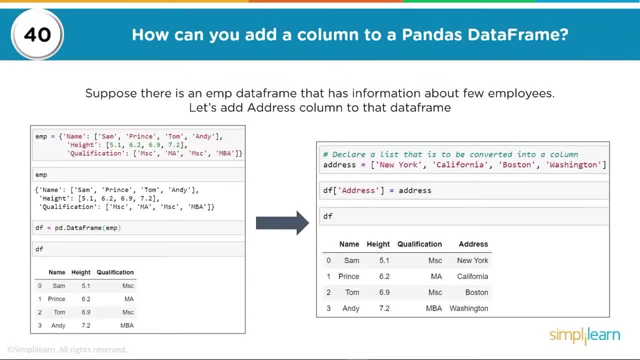 Let's add address column to that data frame And you can see in the left we have our basic data frame. You should know your data frames very well. Basically it looks like an Excel spreadsheet. As you come over here it's really simple. 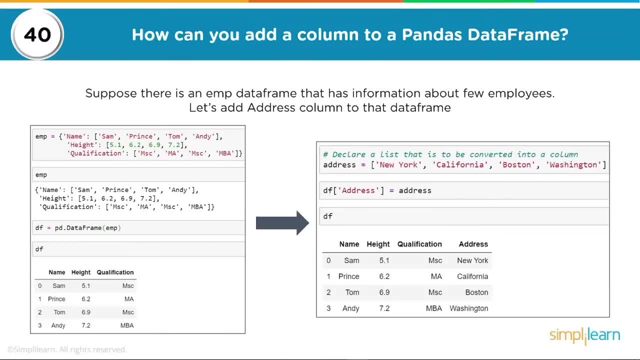 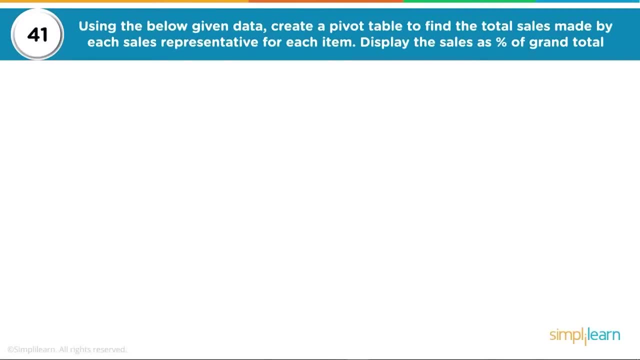 You just do. df of address equals the address. once you've assigned values to the address, Using the below given data: create a pivot table to find the total cells made by each cells represented for each item. Display the cells as a percentage of the grand total. 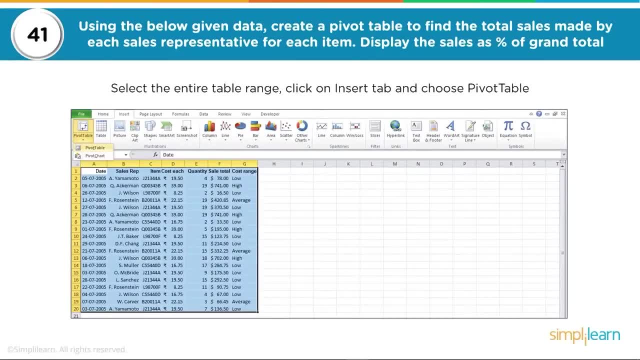 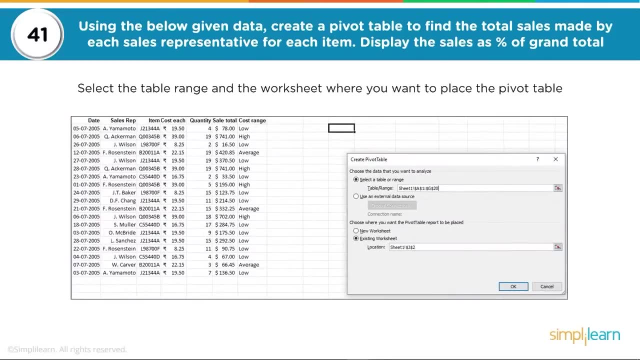 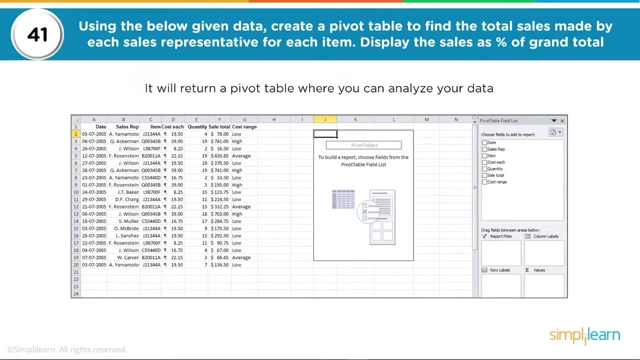 So we're back in Tableau. Select the entire table range, Click on insert tab and choose pivot table. Select the table range and the worksheet where you want to place the pivot table. It will return a pivot table where you can analyze your data. 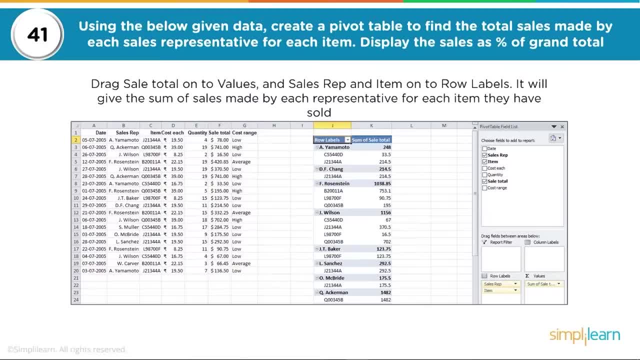 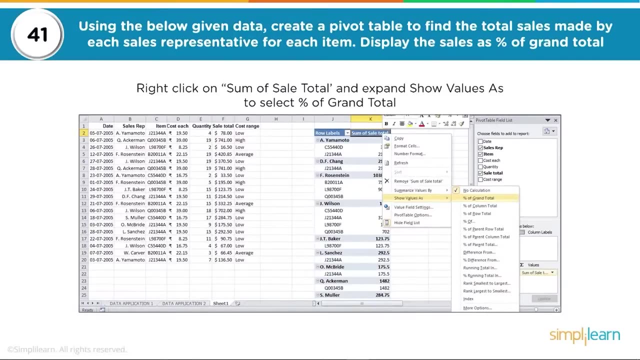 Drag the cell total on the values and cells, rep and item onto row labels. It will give the sum of the cells made by each representative for each item they have sold. And finally, right click on sum of cell total and expand show values as to select percentage of grand total. 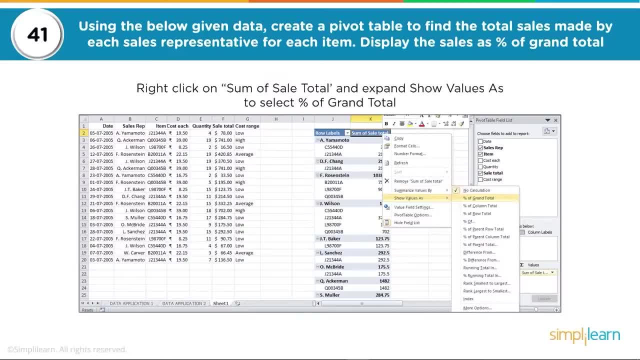 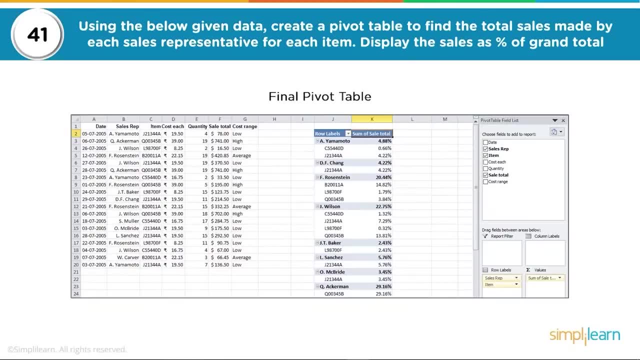 Real important. just to understand what a pivot table is, We're just pivoting it from rows and columns and switching this direction on there And finally we have our final pivot table And you can see the values, rows and sum of total cell. 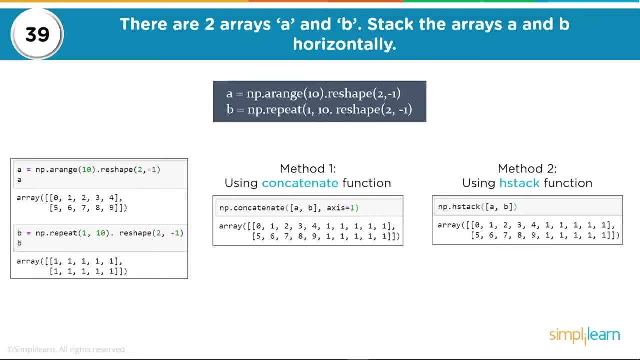 axes equal 1. that is the same as H stack, and in the back end they're still. and in the back end they're still and in the back end they're still identical. they run the same, that's all. identical. they run the same, that's all. 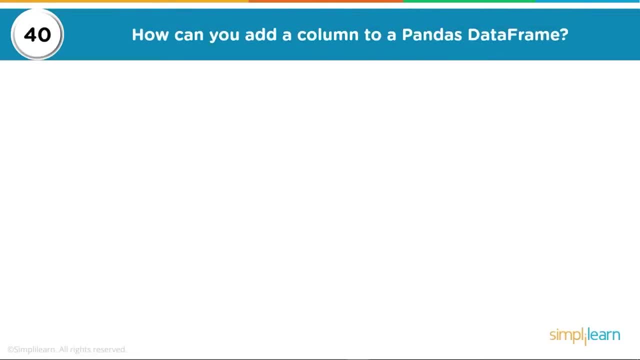 identical. they run the same, that's all. each deck is a concatenate axes equals each deck is a concatenate axes equals each deck is a concatenate axes equals 1. how can you add a column to a pandas 1? how can you add a column to a pandas? 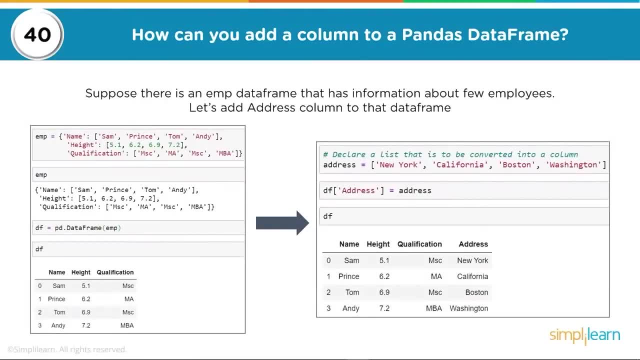 1: how can you add a column to a pandas data frame? suppose there's an imp data data frame. suppose there's an imp data data frame. suppose there's an imp data frame that has information about few frame. that has information about few frame. that has information about few employees. let's add address column to. 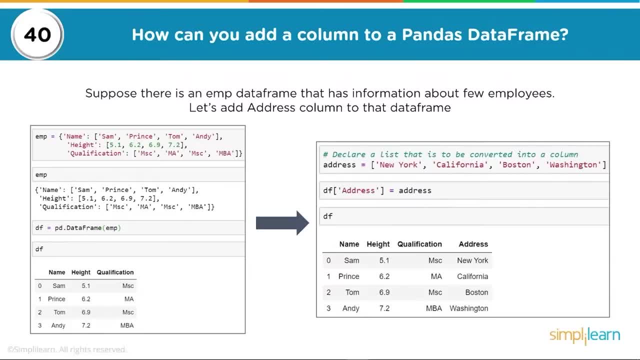 employees. let's add address column to employees. let's add address column to that data frame. and you can see in the that data frame and you can see in the that data frame and you can see in the left, we have our basic data frame. you left, we have our basic data frame, you. 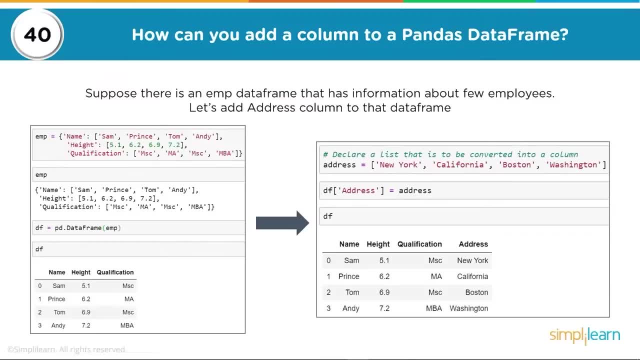 left we have our basic data frame. you should know your data frames very well. should know your data frames very well. should know your data frames very well. basically looks like an Excel. basically looks like an Excel. basically looks like an Excel spreadsheet. as you come over here, it's. 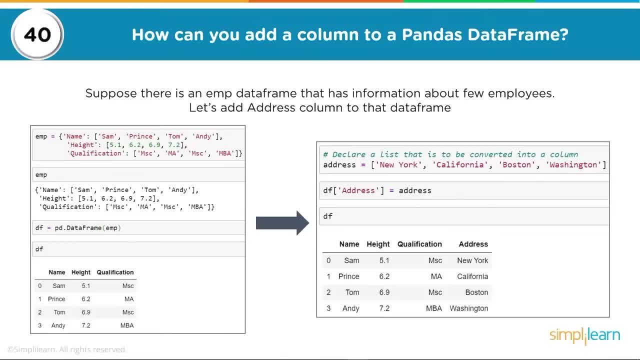 spreadsheet as you come over here. it's spreadsheet as you come over here. it's really simple. you just do DF of address, really simple. you just do DF of address, really simple. you just do: DF of address: equals the address once you've assigned. equals the address once you've assigned. 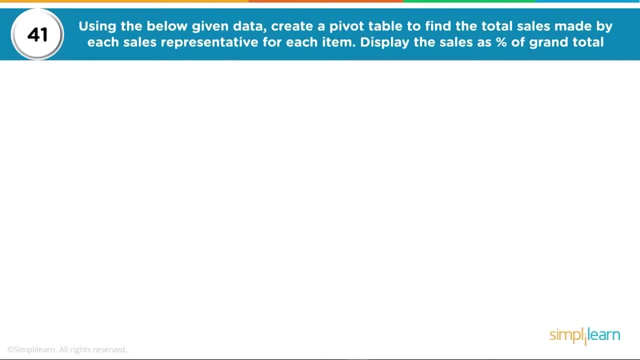 equals the address. once you've assigned values to the address, using the below values to the address. using the below values to the address, using the below given data: create a pivot table to find given data. create a pivot table to find given data. create a pivot table to find the total cells made by each cells. 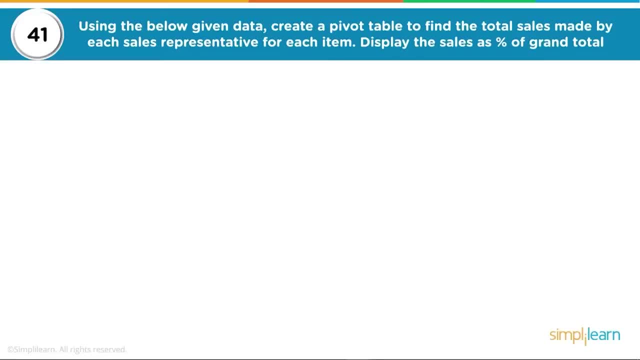 the total cells made by each cells: the total cells made by each cells represented for each item. display the represented for each item. display the represented for each item. display the cells as a percentage of the grand total cells as a percentage of the grand total cells as a percentage of the grand total. so we're back in tab loom. select the. 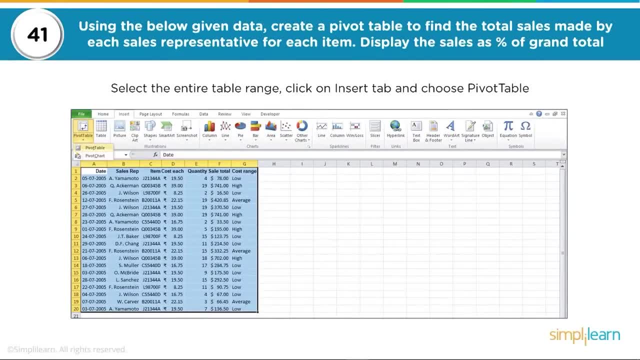 so we're back in tab loom. select the. so we're back in tab loom. select the entire table range. click on insert tab. entire table range. click on insert tab- entire table range. click on insert tab and choose pivot table. select the table. and choose pivot table. select the table. 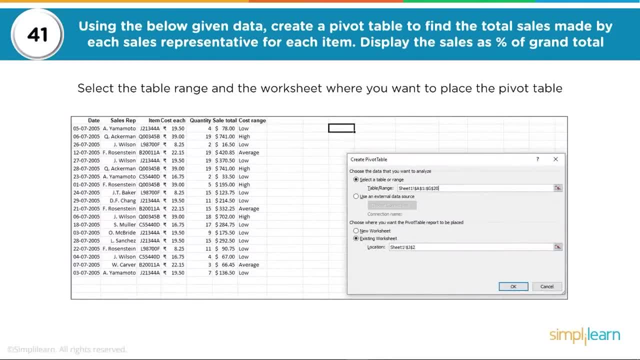 and choose pivot table. select the table range and the worksheet where you want range and the worksheet where you want range and the worksheet where you want to place the pivot table. it will return to place the pivot table. it will return to place the pivot table. it will return a pivot table where you can analyze your. 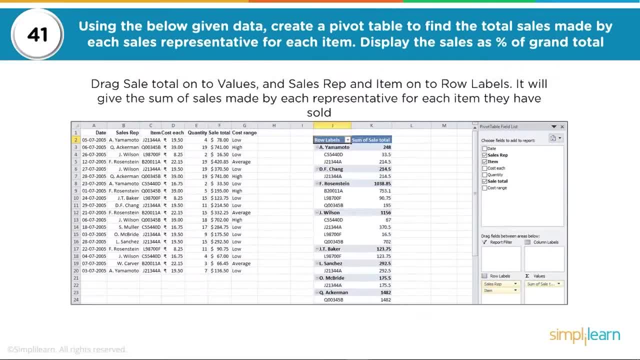 a pivot table where you can analyze your a pivot table where you can analyze your data. drag the cell total on the values data. drag the cell total on the values data. drag the cell total on the values and cells. rep and item onto row. labels and cells. rep and item onto row labels. 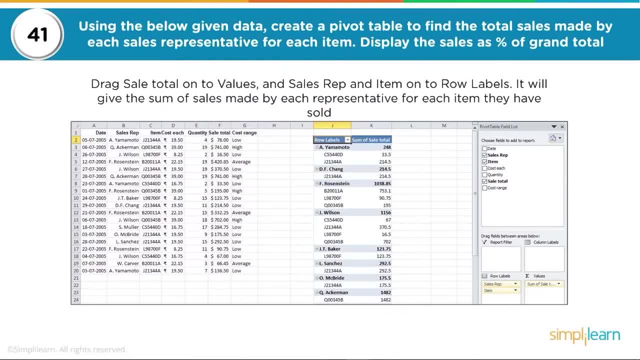 and cells, rep and item onto row labels. it'll give the sum of the cells made by. it'll give the sum of the cells made by. it'll give the sum of the cells made by each representative for each item. they each representative for each item. they each representative for each item they have sold. and finally, right-click on. 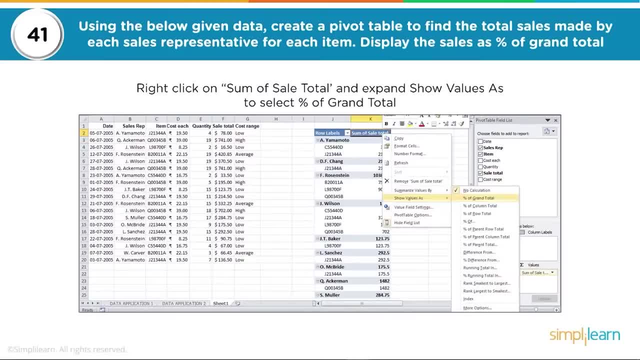 have sold and finally right-click on have sold and finally right-click on sum of cell total and expand: show values as sum of cell total and expand show values as sum of cell total. and expand show values as to select percentage of grand total. to select percentage of grand total. 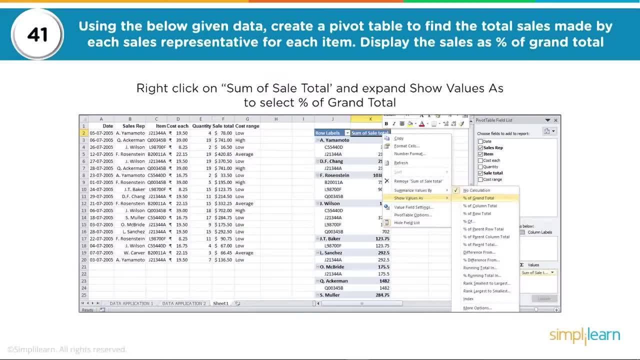 to select percentage of grand total. real important. just understand what a real important. just understand what a real important. just understand what a pivot table is. we're just pivoting it. pivot table is. we're just pivoting it. pivot table is. we're just pivoting it from rows and columns and switching this. 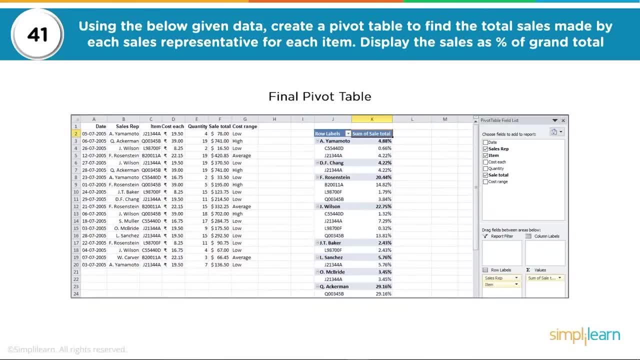 from rows and columns and switching this from rows and columns and switching this direction on there, and finally we have direction on there and finally we have direction on there and finally we have our final pivot table and you can see our final pivot table and you can see. 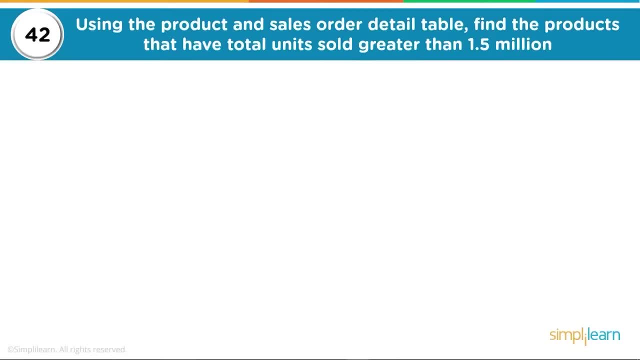 our final pivot table and you can see the values, rules and sum of total sale. the values, rules and sum of total sale. the values, rules and sum of total sale. so we're going to go ahead and take a. so we're going to go ahead and take a. 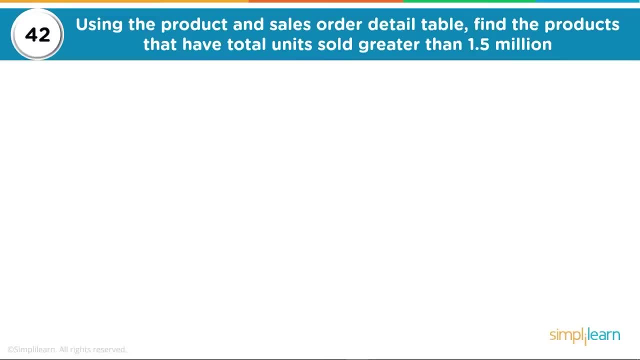 so we're going to go ahead and take a product table. this is off of an SQL, so product table: this is off of an SQL. so product table: this is off of an SQL. so we're gonna do some SQL here and we're. we're gonna do some SQL here and we're. 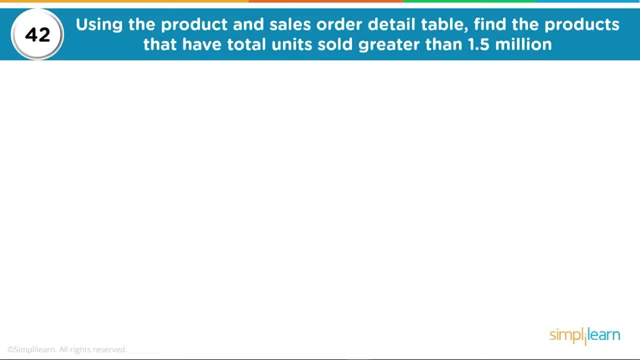 we're gonna do some SQL here and we're gonna use the product and sales order. gonna use the product and sales order. gonna use the product and sales order detail table. find the products that have detail table. find the products that have detail table. find the products that have total units sold greater than 1.5 million. 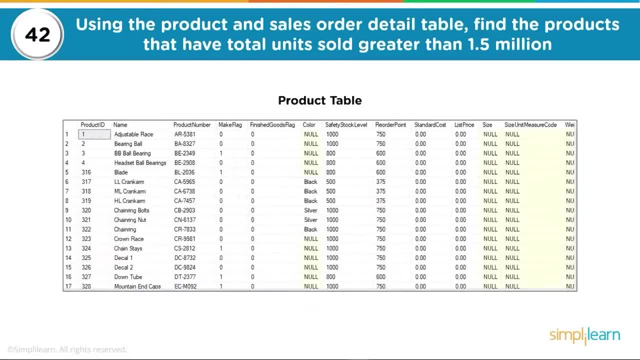 total units sold greater than 1.5 million. total units sold greater than 1.5 million. and here's our sales order detail table. and here's our sales order detail table. and here's our sales order detail table. so we have a product table and a sales. 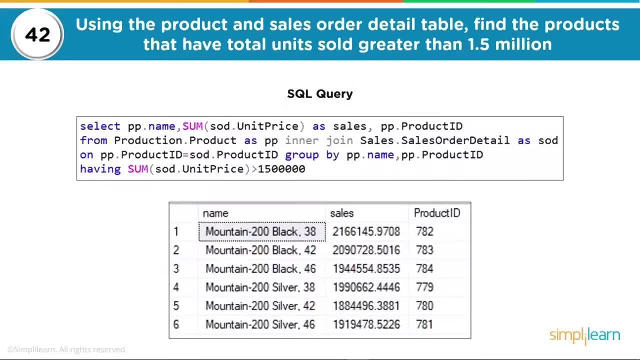 so we have a product table and a sales. so we have a product table and a sales order detail table, two separate tables in order detail table, two separate tables in order detail table, two separate tables in the database. and we're gonna do is put the database and we're gonna do is put. 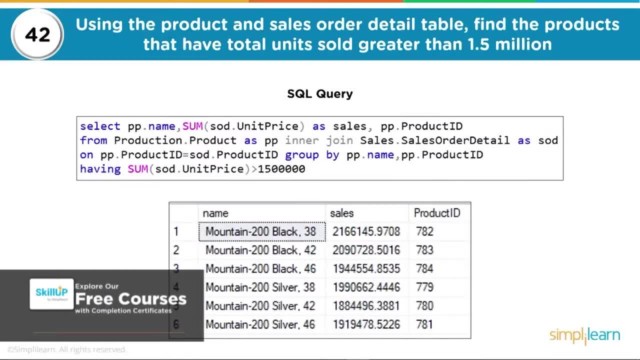 the database and we're gonna do is put together the SQL query. we want to select together the SQL query. we want to select together the SQL query. we want to select: PP name- some sod unit price as cells and. PP name- some sod unit price as cells and. 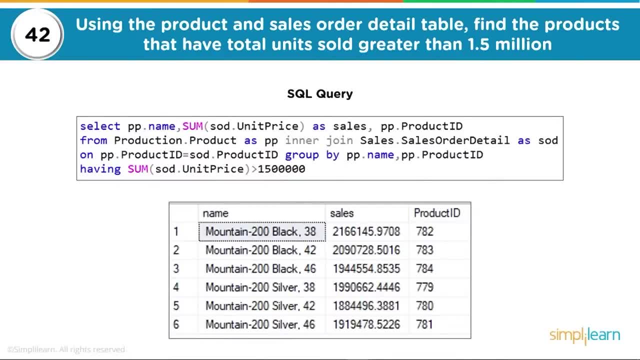 PP name some sod unit price as cells and then we have our PP product ID. from then we have our PP product ID. from then we have our PP product ID from production product as PP interjoin cells. production product as PP interjoin cells. production product as PP interjoin cells dot. sales order detail as sod on PP. 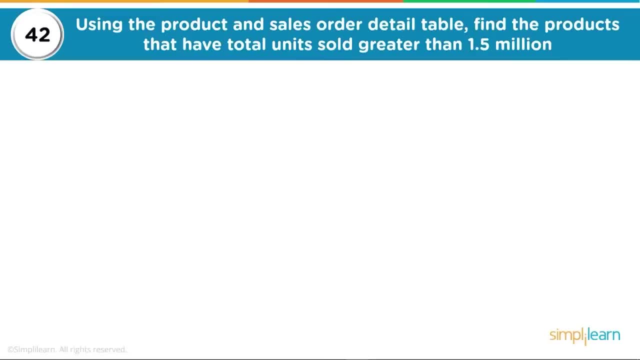 So we're going to go ahead and take a product table. This is off of an SQL, So we're going to do some SQL here And we're going to use the product and sales order detail table. Find the products that have total units sold greater than 1.5 million. 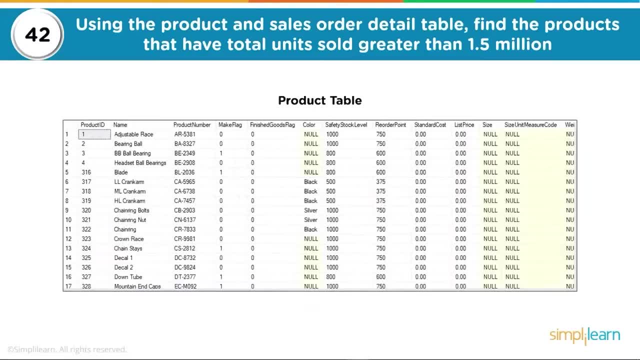 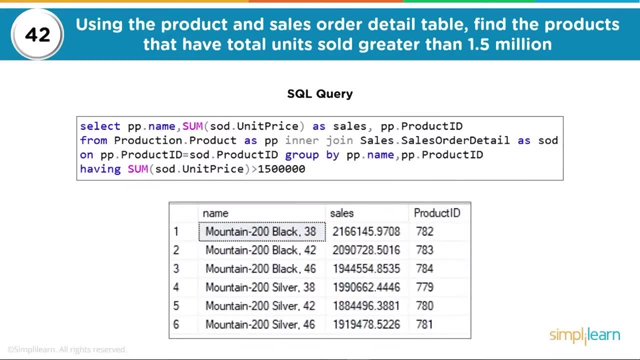 And here's our sales order detail table. So we have a product table and a sales order detail table, two separate tables in the database, And what we're going to do is put together the SQL query. We want to select PP, name, sum, sod, unit, price as cells. 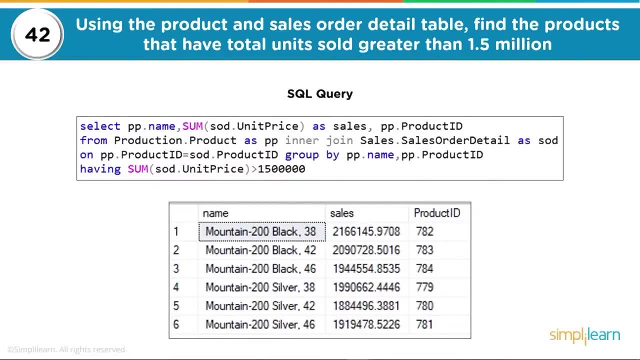 And then we have our PP dot product ID from production product as PP inner join Sales dot sales order detail as sod on PP product ID equals sod dot product ID Group by PP dot name comma. PP dot product ID having a sum of sod dot unit price greater than the 150 million there. 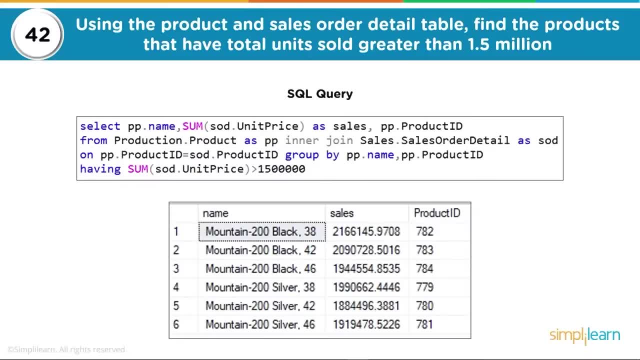 That's a mouthful. And again these SQL queries. they start looking really crazy until you just break them apart and do them step by step. And what we're looking for is the inner join. and how did you do the group by? That's really wanting to know how do you do this inner join? 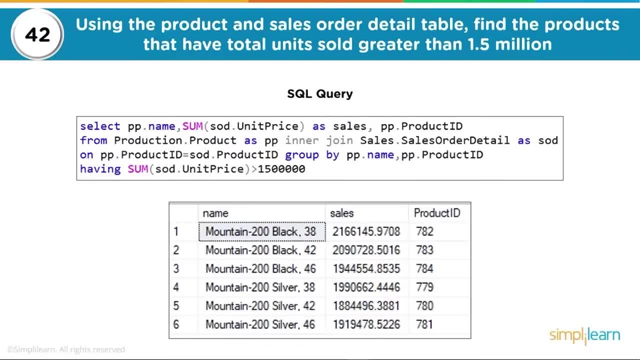 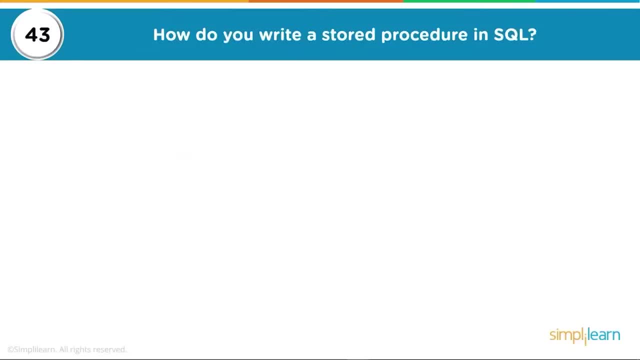 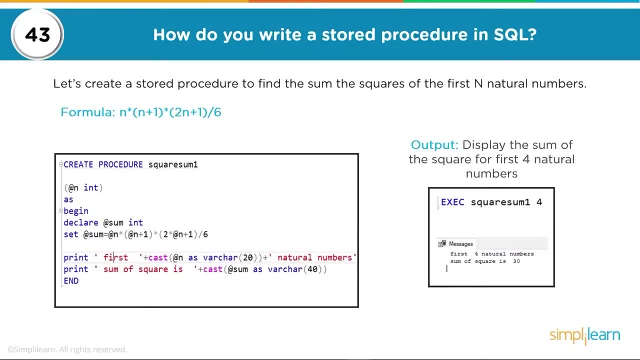 This comes up so much in SQL. How do you pull in the ID from one chart and the information from another chart and the sum totals on that chart? How do you write a stored procedure in SQL? Let's create a stored procedure to find the sum, the squares, of the first n natural numbers. 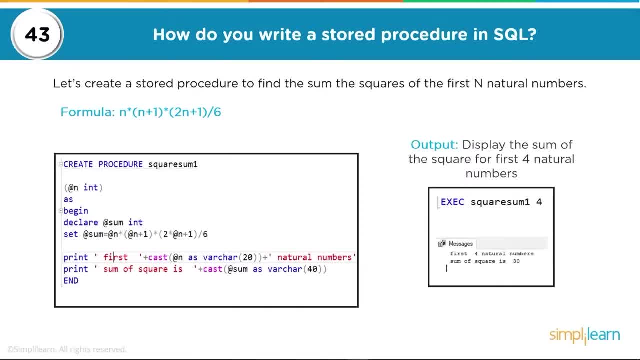 So here we have our formula: n times n plus 1 times 2n plus 1 over 6.. And you can see from the command prompt or the setup you have, depending on what your login is. The command is create procedure: square sum 1.. 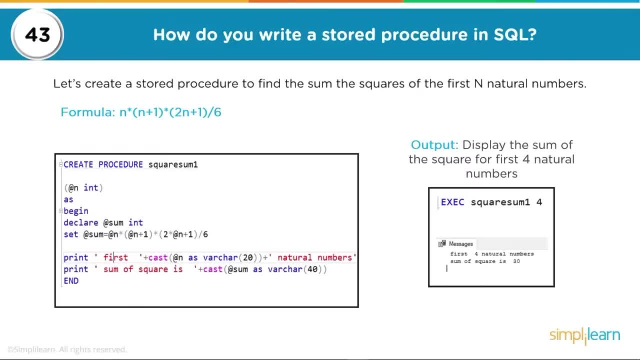 Declare our variable at n of integer as begin. Then we're going to declare the sum of integer Set sum equals n times n plus 1.. Plus 2 times n plus 1 over 6.. And then, of course, we can go ahead and print those out. 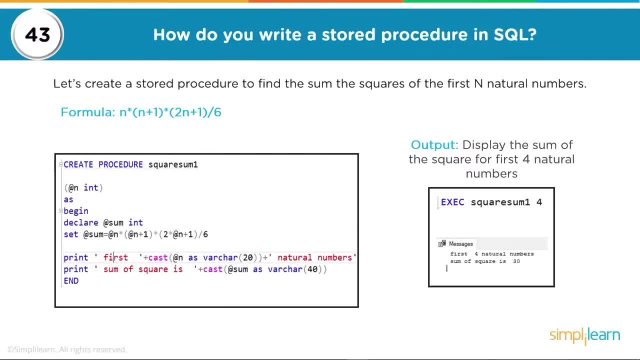 Print: first cast embersign n or our variable as a variable character: 20 natural numbers. Print the sum of the square is cast the at sum as variable character: 40 int. Then we do the output Display the sum of the square for first four natural numbers. 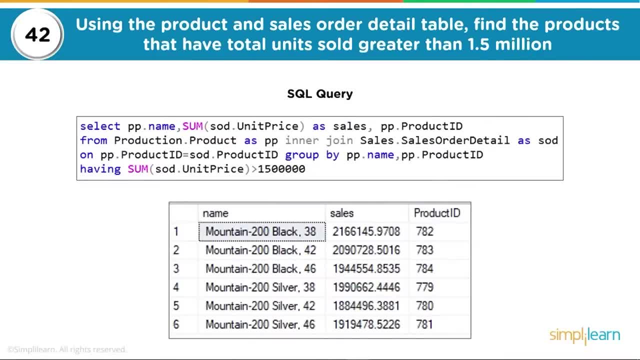 dot sales order detail as sod on PP. dot sales order detail as sod on: PP. product ID: equals sod product ID group by product ID: equals sod product ID group by product ID: equals sod product ID group by PP name comma: PP product ID having a PP name comma: PP product ID having a. 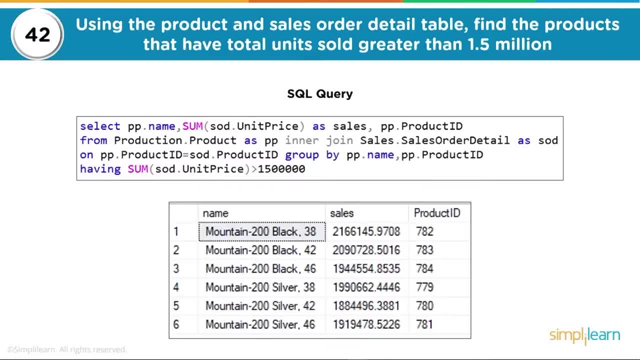 PP name, comma, PP product ID having a sum of sod unit price greater than the sum of sod unit price greater than the sum of sod unit price greater than the hundred and fifty million. there, that's a hundred and fifty million. there, that's a hundred and fifty million. there, that's a mouthful. and again these SQL queries. 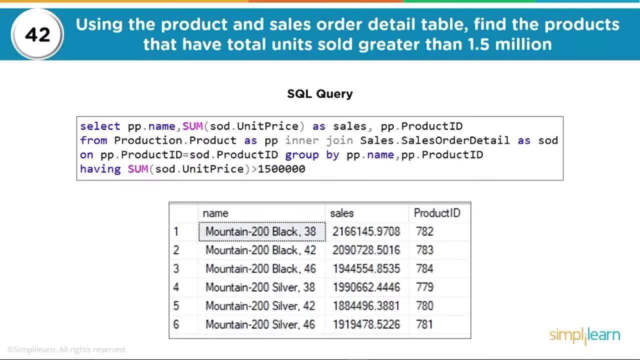 mouthful and again these SQL queries. mouthful and again these SQL queries. they start looking really crazy. until they start looking really crazy, until they start looking really crazy, until you just break them apart and do them. you just break them apart and do them. you just break them apart and do them step by step, and whether we're looking 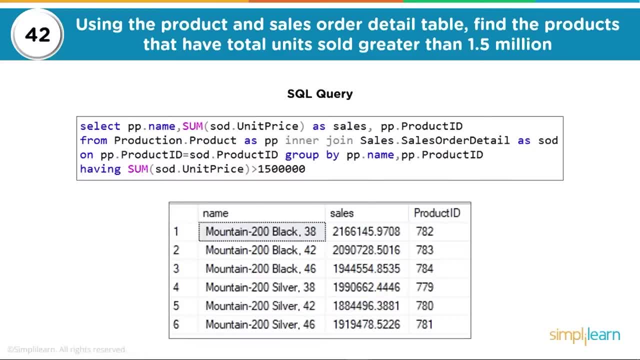 step by step and whether we're looking step by step and whether we're looking for: is the inner join and how did you do for? is the inner join and how did you do for? is the inner join and how did you do the group by this, really one of they? 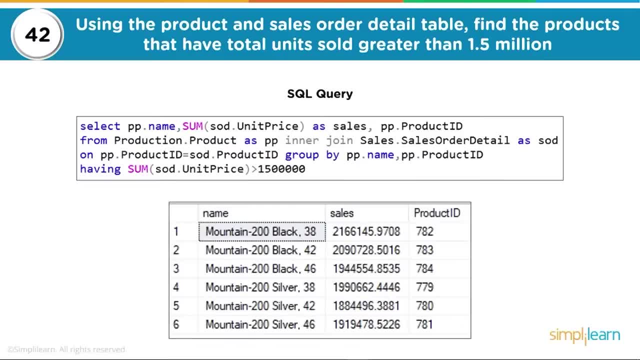 the group by this, really one of they. the group by this, really one of they. know how do you do this inner join this? know, how do you do this inner join this? know how do you do this inner join? this comes up so much in SQL. how do you pull? 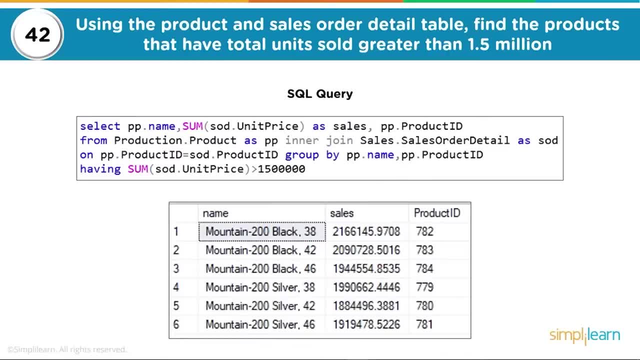 comes up so much in SQL. how do you pull? comes up so much in SQL. how do you pull in the ID from one chart and the in the ID from one chart and the in the ID from one chart and the information from another chart and the information from another chart and the? 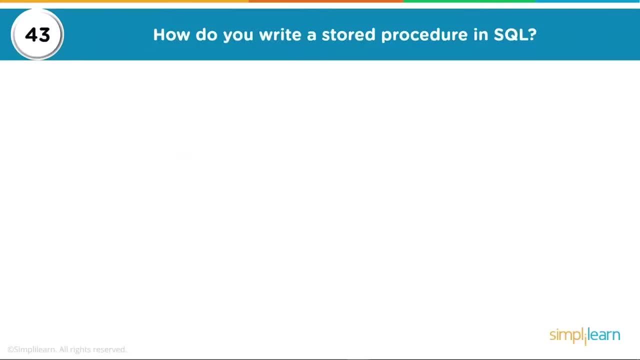 information from another chart and the sum totals on that chart. how do you write sum totals on that chart? how do you write sum totals on that chart? how do you write a stored procedure in SQL? let's a stored procedure in SQL. let's a stored procedure in SQL. let's create a stored procedure to find the. 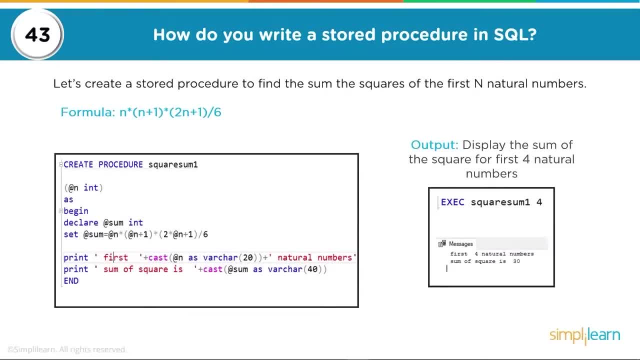 create a stored procedure to find the. create a stored procedure to find the sum. the squares are the first in natural sum. the squares are the first in natural sum. the squares are the first in natural numbers. so here we have our formula in numbers. so here we have our formula in. 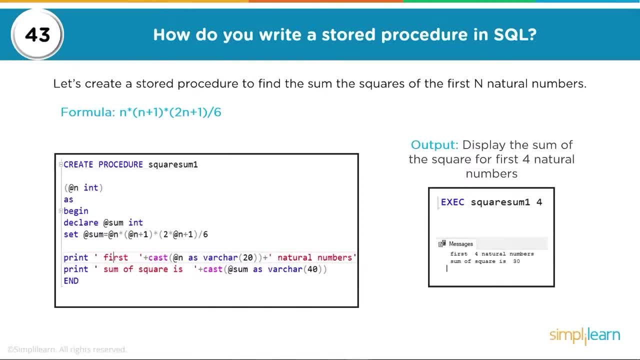 numbers. so here we have our formula in times n plus 1 times 2 n plus 1 over 6 times n plus 1 times 2 n plus 1 over 6 times n plus 1 times 2 n plus 1 over 6, and you can see from the command prompt. 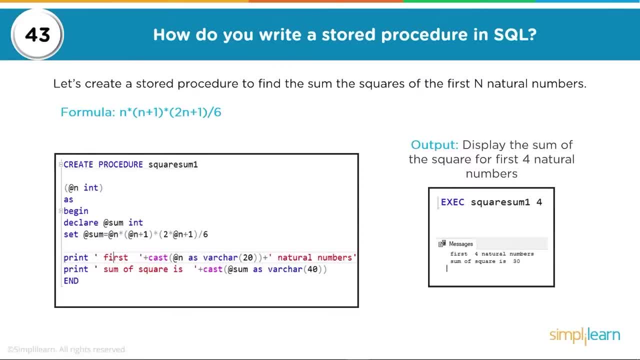 and you can see from the command prompt. and you can see from the command prompt, or the setup you have we're depending on, or the setup you have we're depending on, or the setup you have. we're depending on what your login is. the command is create. 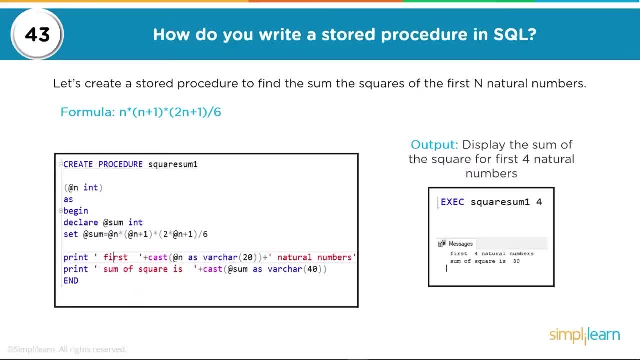 what your login is. the command is: create what your login is. the command is create procedure square sum 1. declare our procedure square sum 1. declare our procedure square sum 1. declare our variable at n of integer as begin then. variable at n of integer as begin then. 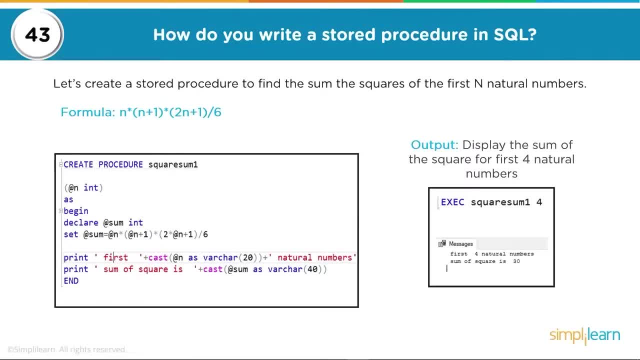 variable at n of integer as begin, then we're going to declare the sum of. we're going to declare the sum of. we're going to declare the sum of: integer set sum equals n times n plus 1. integer set sum equals n times n plus 1. 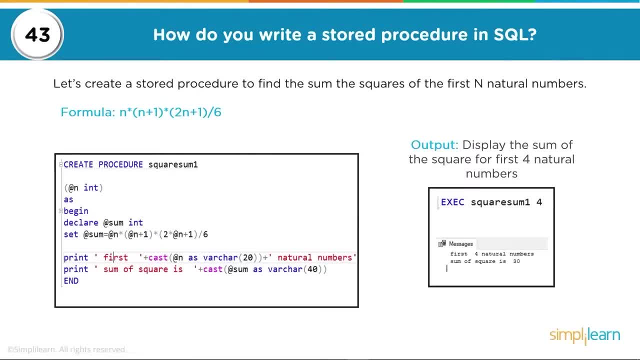 integer set sum equals n times n plus 1 plus 2 times n plus 1 over 6, and then of plus 2 times n plus 1 over 6, and then of plus 2 times n plus 1 over 6, and then, of course, we can go ahead and print those. 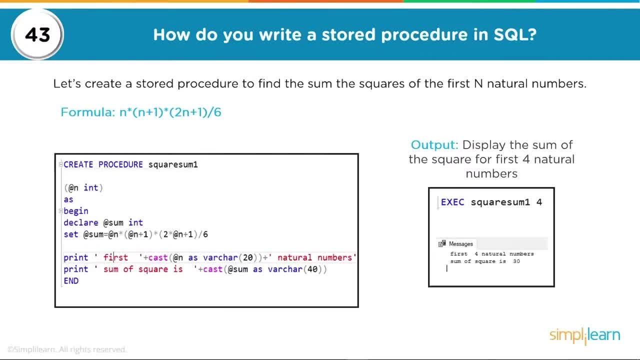 course we can go ahead and print those. course we can go ahead and print those out print first cast ember sign in or a out print first cast ember sign in or a out print first cast ember sign in or a variable as a variable character: 20. variable as a variable character: 20. 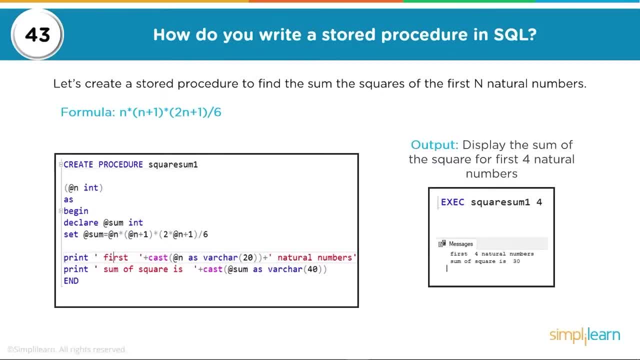 variable as a variable character: 20 natural numbers. print the sum of the natural numbers. print the sum of the natural numbers. print the sum of the square is cast. the at sum as a variable square is cast. the at sum as a variable square is cast. the at sum as a variable character: 40 int. then we do the output. 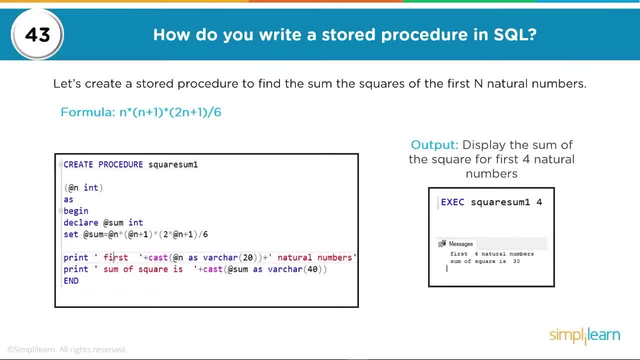 character 40 int. then we do the output character 40 int. then we do the output. display the sum of the square for first. display the sum of the square for first. display the sum of the square for first. four natural numbers. we have execute. four natural numbers. we have execute. 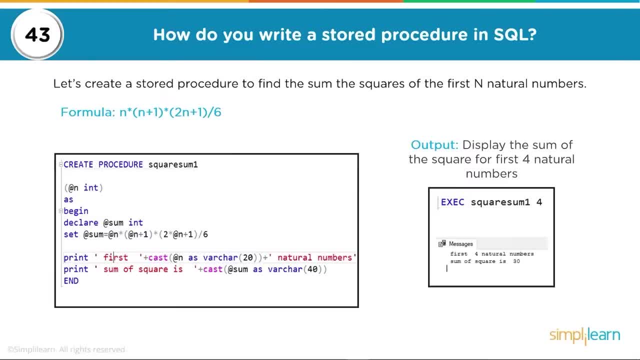 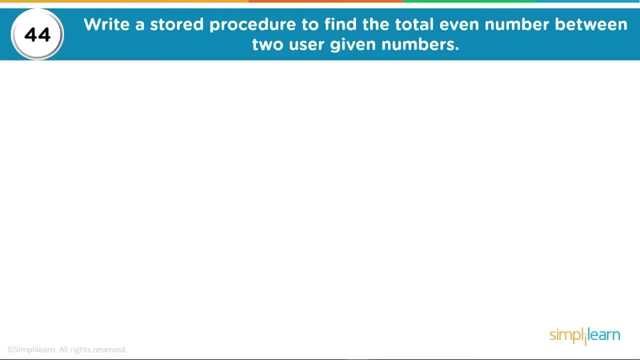 We have execute square sum 1. And then we're going to put in 4. And you can see here where it brings up the first four natural numbers. Sum of square is 30.. Write a stored procedure to find the total even number between two user given numbers. 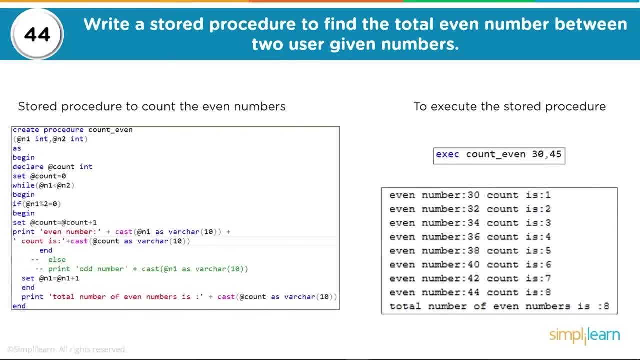 A couple of things to note here. First, we go ahead and create our procedure. You have your two different variables, The n1, n2.. And we go ahead and begin. We're going to declare our variable count as an integer. We're going to set count equal to 0. 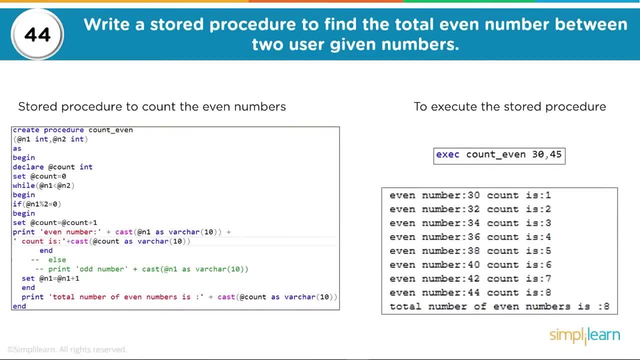 We have, while n is less than n2.. We're going to begin, And if n1 remainder, 2 equals 0. So we're going to divide it by 2.. Even number: Begin. We're going to set the count equal to count plus 1.. 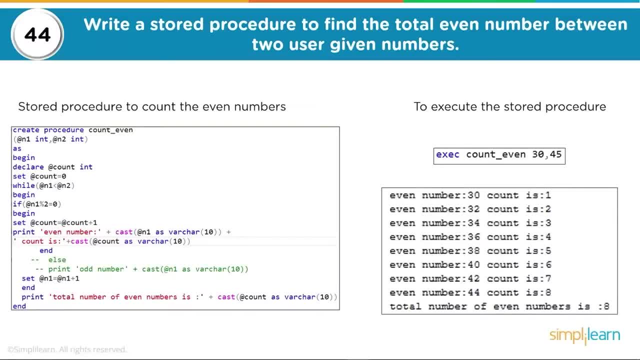 We're going to print even number plus cast n as a variable character 10 for printing Count is plus cast variable count as variable character 10 int. Else print odd number plus cast variable number 1 as variable character 10 int. And then we go ahead and set the increment our variable 1 up 1.. 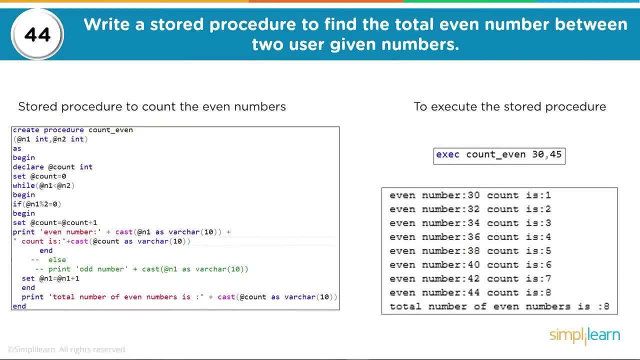 So it goes from n1 all the way to n2.. And it'll print the total number of even numbers And you can see here we went ahead and executed it. We're going to count the even numbers between 30 and 45.. 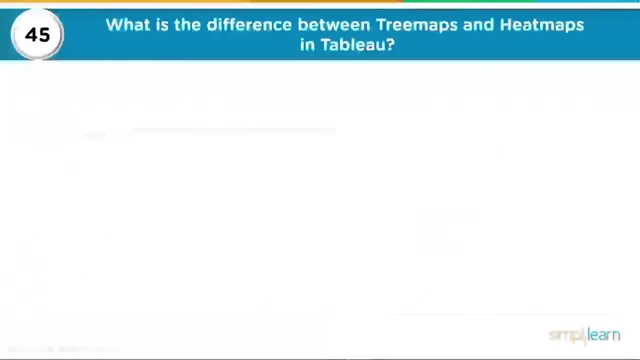 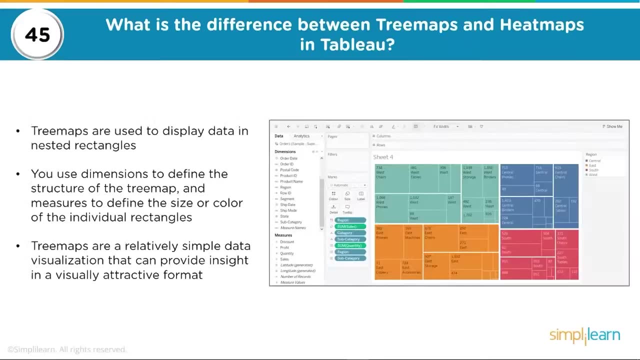 And you can just see it goes all the way down to 8.. What is the difference between tree maps and heat maps in Tableau? Now, if you've worked in Python and other programmings, You should automatically know what a heat map is. 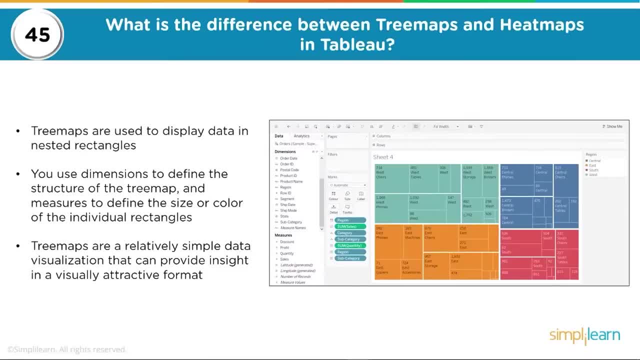 But a tree map, are used to display data in nested rectangles. You use dimensions to define the structure of the tree map And measure to define the size or color of individual rectangles. Tree maps are relatively simple data visualization That can provide insight in a visually attractive format. 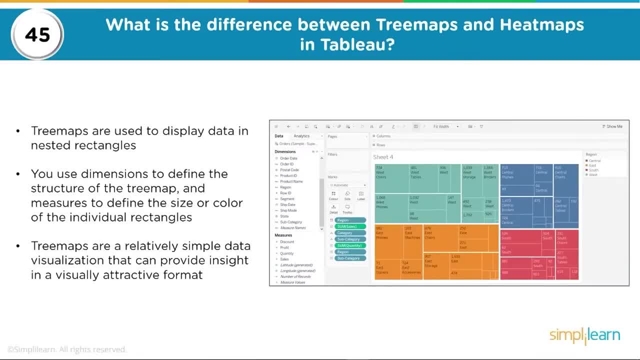 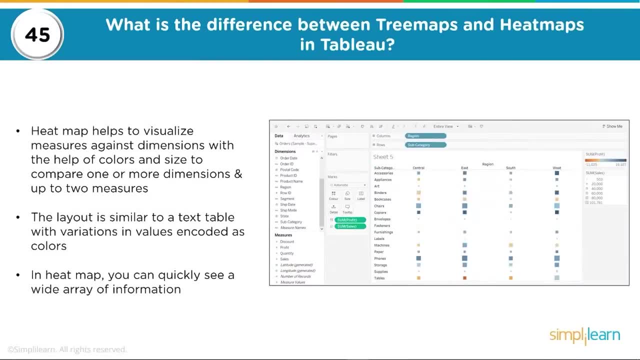 And again you can see the squares over here. This is our tree map over here with the. Each block also has this information inside of it. It's different blocks. A heat map helps to visualize measures against dimensions With the help of colors and size. 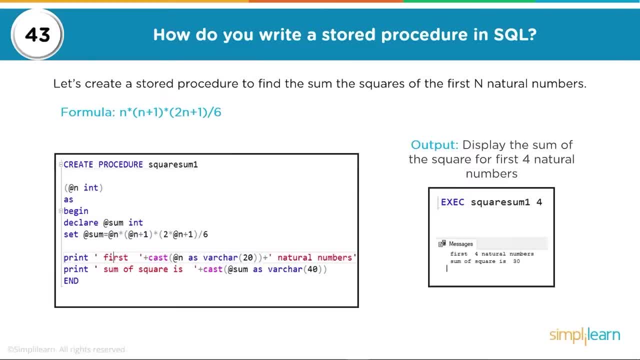 four natural numbers we have. execute square sum 1 and then we're gonna put in square sum 1, and then we're gonna put in square sum 1 and then we're gonna put in 4, and you can see here where it brings 4, and you can see here where it brings. 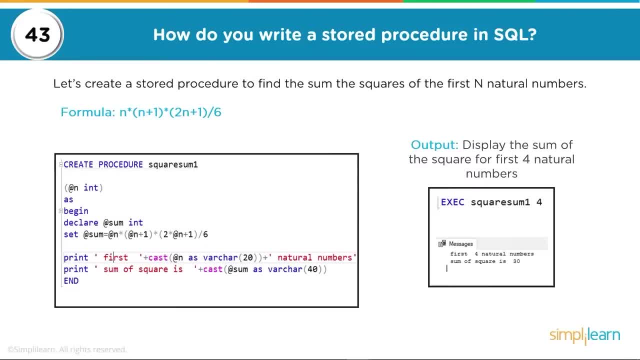 4 and you can see here where it brings up the first four natural numbers. sum of up the first four natural numbers. sum of up the first four natural numbers. sum of square is 30. write a store procedure to: square is 30. write a store procedure to. 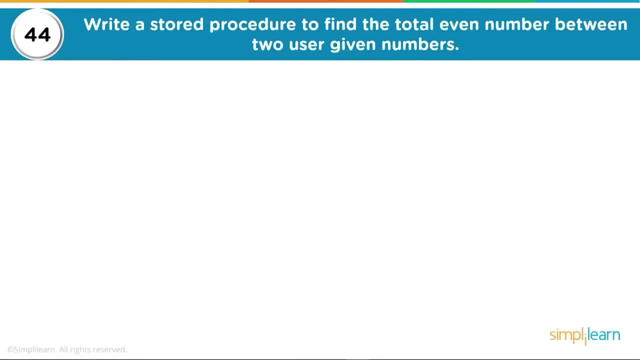 square is 30. write a store procedure to find the total even number between two. find the total even number between two. find the total even number between two user given numbers. a couple of things to user given numbers. a couple of things to user given numbers. a couple of things to know here. first we go ahead and create. 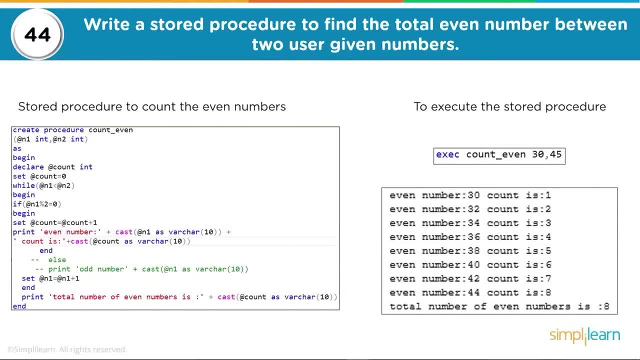 know here first we go ahead and create. know here first, we go ahead and create our procedure. you have your two, our procedure. you have your two, our procedure. you have your two different variables, the n1 in two and we different variables: the n1 in two and we. 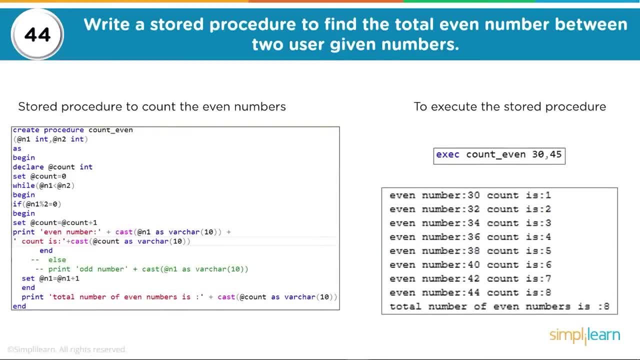 different variables, the n1 in two, and we go ahead and begin. we're going to go ahead and begin. we're going to go ahead and begin. we're going to declare our variable count as an integer. declare our variable count as an integer. declare our variable count as an integer. we're gonna set count equal to zero and 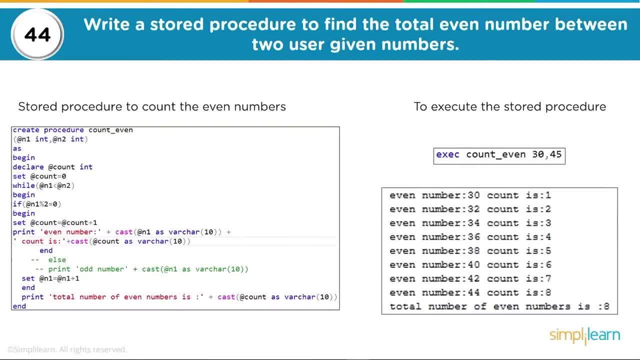 we're gonna set count equal to zero, and we're gonna set count equal to zero, and then we have: while n is less than n2, then we have. while n is less than n2, then we have. while n is less than n2, we're going to begin, and if n1 remainder, 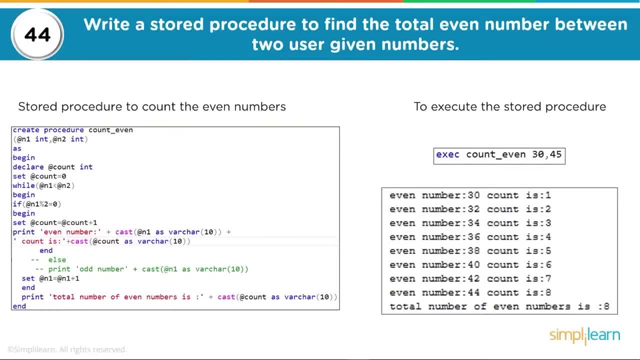 we're going to begin. and if n1 remainder, we're going to begin. and if n1 remainder 2 equals 0, so we're going to divided by 2 equals 0. so we're going to divided by 2 equals 0, so we're going to divided by 2, even number: begin: we're going to set. 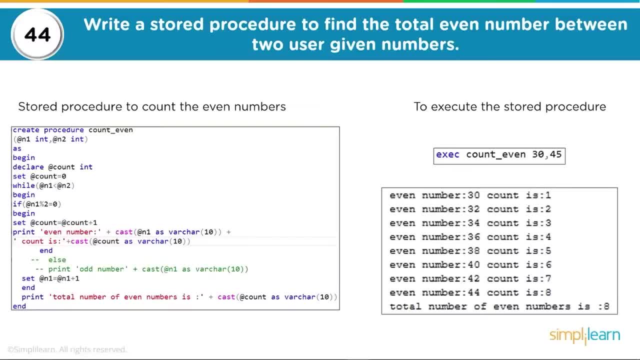 2 even number. begin. we're going to set 2- even number. begin. we're going to set the count equal to count plus 1. we're the count equal to count plus 1. we're the count equal to count plus 1. we're gonna print even number plus cast in as: 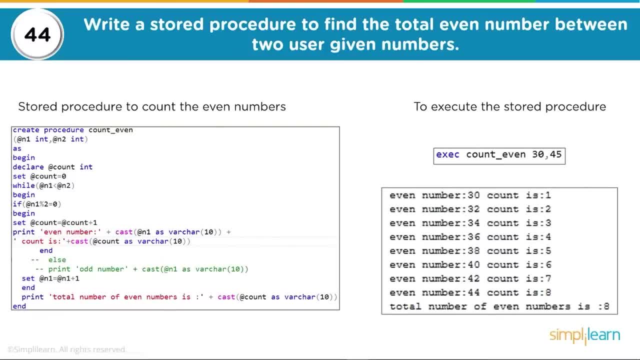 gonna print even number plus cast in as. gonna print even number plus cast in as a variable character: 10 for printing a variable character. 10 for printing a variable character. 10 for printing. count is plus cast. variable count as. count is plus cast. variable count as. 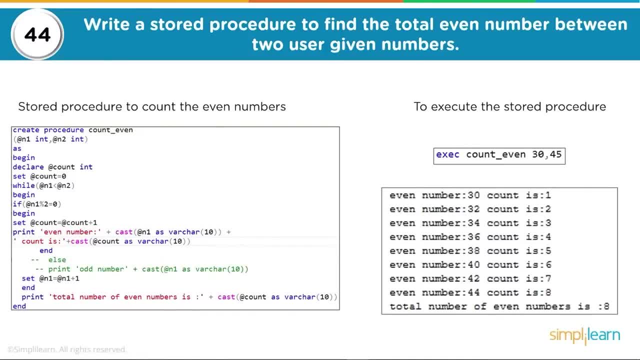 count is plus cast variable count as variable character 10. end, else print odd variable character 10. end else print odd variable character 10. end, else print odd number plus cast variable number 1 as number, plus cast variable number 1 as number, plus cast variable number 1 as variable character 10, and then we go. 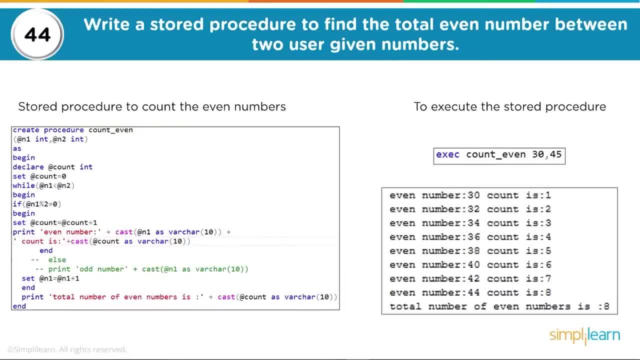 variable character 10 and then we go variable character 10 and then we go ahead and set the increment our variable ahead and set the increment our variable ahead and set the increment our variable 1 up 1, so that goes from n1 all the way. 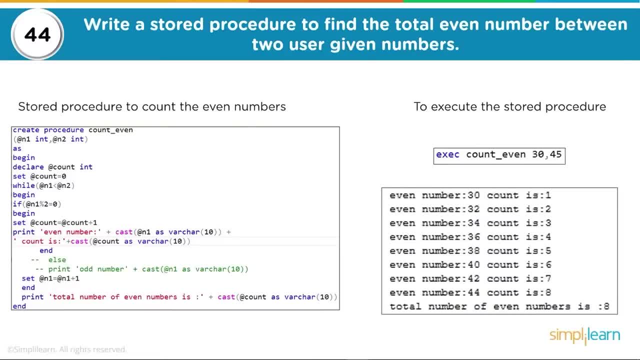 1 up 1, so that goes from n1 all the way 1 up 1, so that goes from n1 all the way to n2. it'll print the total number of to n2. it'll print the total number of to n2. it'll print the total number of even numbers and you can see here we 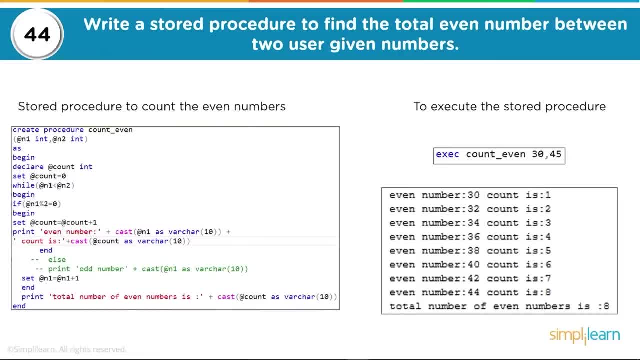 even numbers and you can see here we even numbers and you can see here we went ahead and executed it. we're going, went ahead and executed it. we're going, went ahead and executed it. we're going to count the even numbers between 30 and to count the even numbers between 30 and. 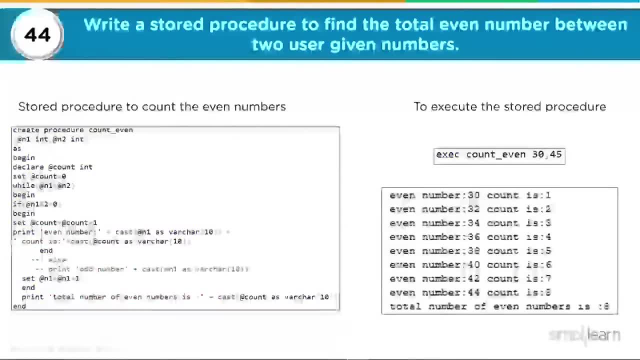 to count the even numbers between 30 and 45, and you see it goes all the way down 45. and you see it goes all the way down 45, and you see it goes all the way down to 8. what is the difference between tree? 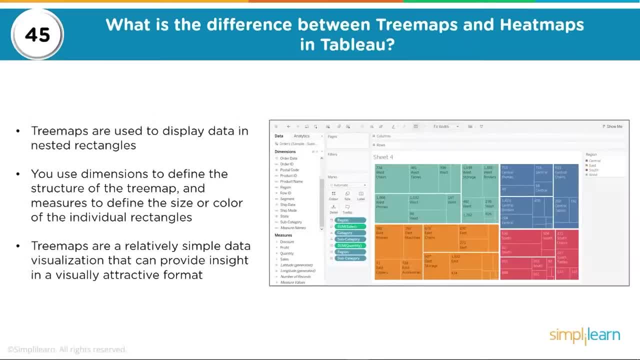 to 8? what is the difference between tree to 8? what is the difference between tree maps and heat maps in tableau now, if maps and heat maps in tableau now, if maps and heat maps in tableau now, if you're worked in Python other, you're worked in Python other. 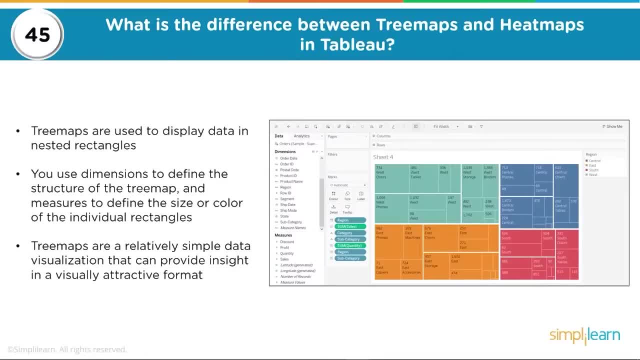 you're worked in Python other programmings, you should automatically programmings. you should automatically programmings. you should automatically know what a heat map is but a tree map. know what a heat map is but a tree map. know what a heat map is but a tree map. are used to display data in nested 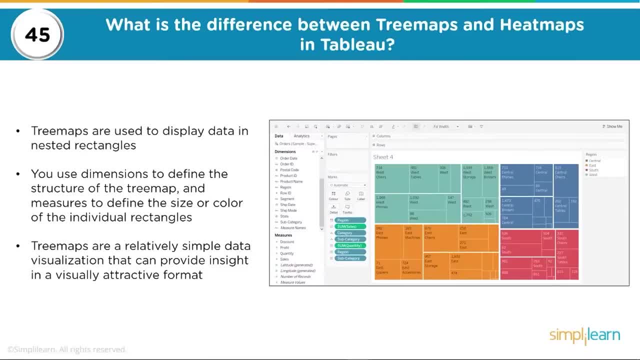 are used to display data in nested are used to display data in nested rectangles. you use dimensions to define rectangles. you use dimensions to define rectangles. you use dimensions to define the structure of the tree map and measure the structure of the tree map and measure the structure of the tree map and measure to define the size or color of. 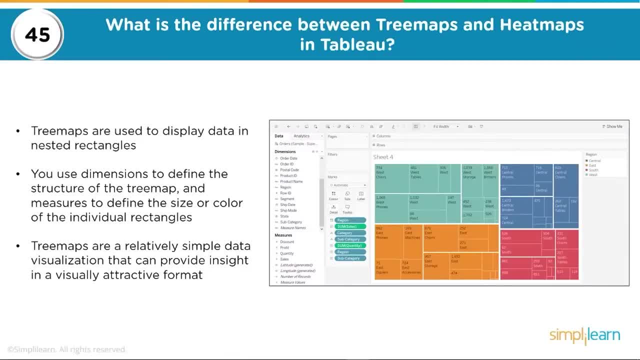 to define the size or color of. to define the size or color of individual rectangles tree maps are a individual rectangles tree maps are a individual rectangles tree maps are a relatively simple data visualization. that relatively simple data visualization, that relatively simple data visualization that can provide insight in a visually 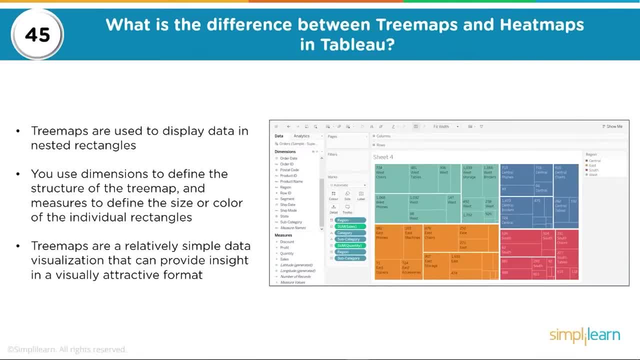 can provide insight in a visually can provide insight in a visually attractive format. and again you can see attractive format. and again you can see attractive format. and again you can see the squares over here. this is our tree, the squares over here, this is our tree, the squares over here, this is our tree map over here, with the each block also. 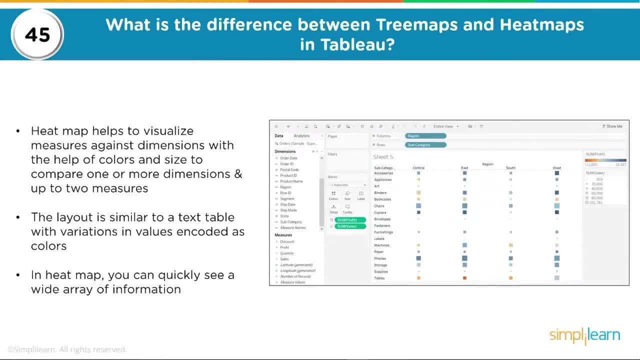 map over here with the each block. also map over here with the each block. also has this information inside of its. has this information inside of its. has this information inside of its different blocks? a heat map helps to different blocks. a heat map helps to different blocks. a heat map helps to visualize measures against dimensions. 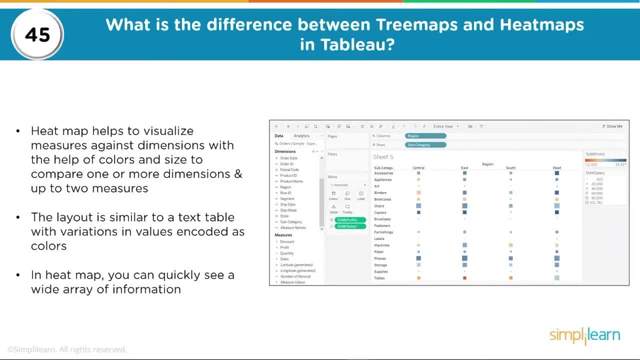 visualize measures against dimensions. visualize measures against dimensions with the help of colors and size. to with the help of colors and size. to with the help of colors and size, to compare one or more dimensions and up to compare one or more dimensions. and up to compare one or more dimensions and up to two measures. the layout is similar to a. 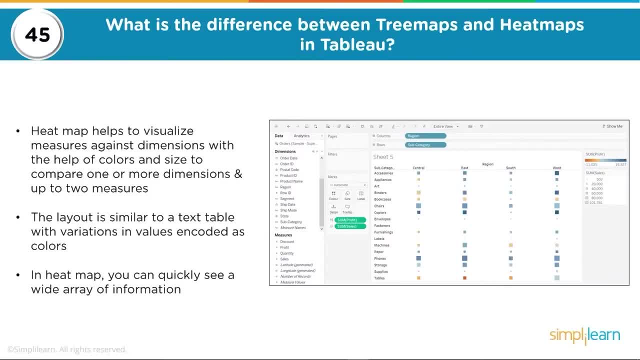 two measures. the layout is similar to a two measures. the layout is similar to a text table with variations in values. text table with variations in values. text table with variations in values encoded as colors in heat map. you can encoded as colors in heat map. you can encoded as colors in heat map. you can quickly see a wide array of information. 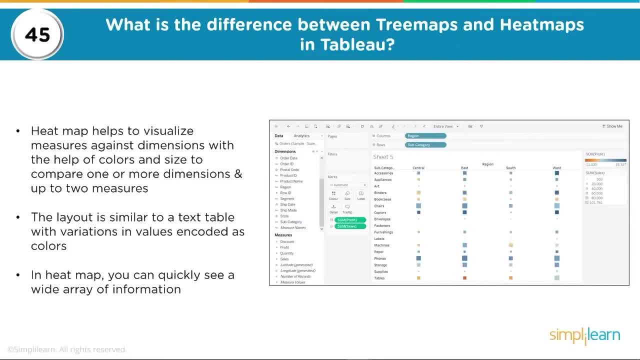 quickly see a wide array of information, quickly see a wide array of information, and in this one you can see they use the and in this one you can see they use the and in this one you can see they use the colors to denote one thing, and the size. 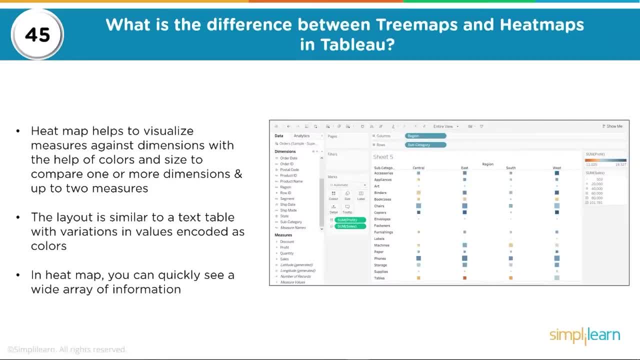 colors to denote one thing. and the size colors to denote one thing. and the size of the little square to denote something of the little square. to denote something of the little square to denote something else. a lot of times you can even graph else. a lot of times you can even graph. 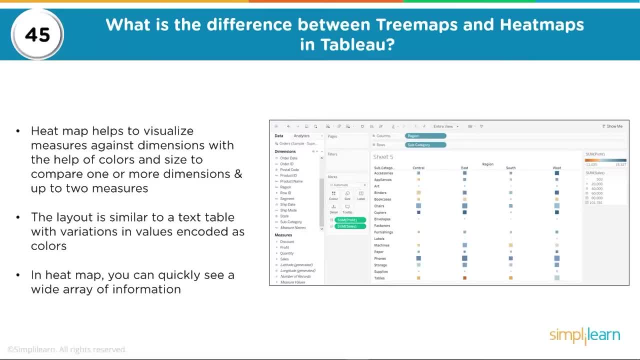 else. a lot of times you can even graph this into a three-dimensional graph with this into a three-dimensional graph with this, into a three-dimensional graph with other data, so it pops out. but again a other data, so it pops out. but again a other data. so it pops out, but again a heat map is the color and the size using. 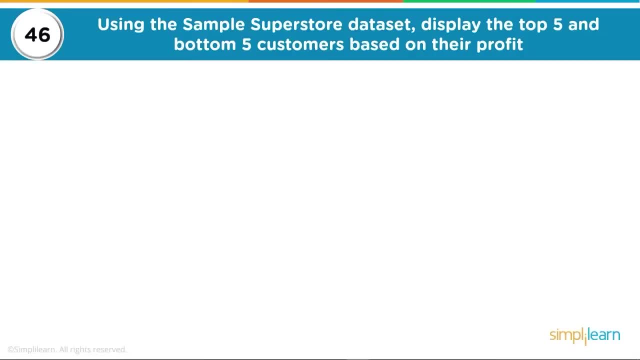 heat map. is the color and the size using heat map. is the color and the size using the sample superstore data set display. the sample superstore data set. display the sample superstore data set. display the top five and bottom five customers. the top five and bottom five customers. 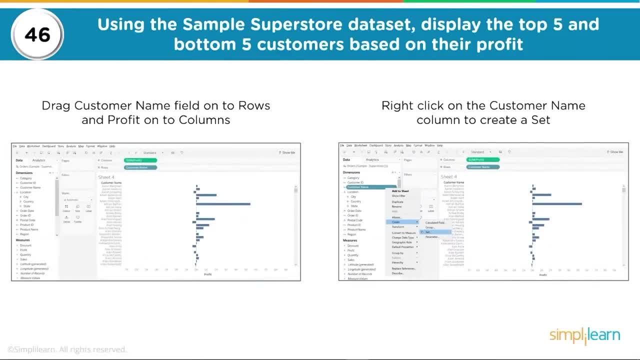 the top five and bottom five customers based on their profit. so you start by based on their profit. so you start by based on their profit. so you start by dragging the customer name filled on to dragging the customer name filled on to. dragging the customer name filled on to rows and profit on columns right-click. 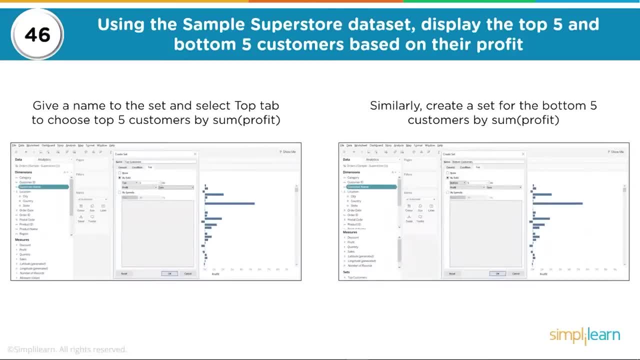 rows and profit on columns. right-click rows and profit on columns. right-click on the customer name column to create a. on the customer name column to create a. on the customer name column to create a set. give a name to the set and select set. give a name to the set and select. 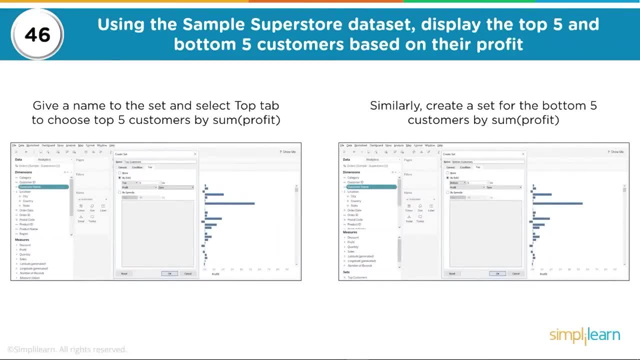 set. give a name to the set and select top tab to choose top five customers by top tab. to choose top five customers by top tab. to choose top five customers by some profit. similarly, create a set for some profit. similarly, create a set for some profit. similarly, create a set for the bottom five customers by some profit. 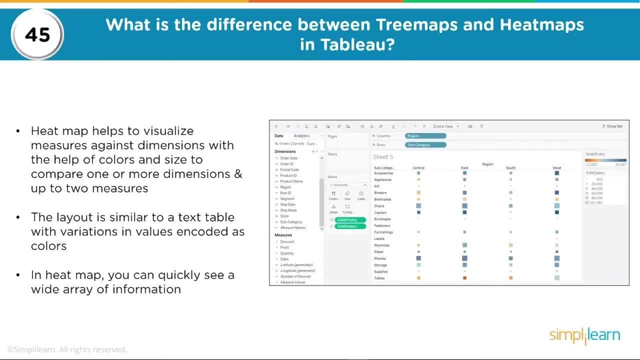 To compare one or more dimensions and up to two measures. The layout is similar to a text table With variations in values encoded as colors. In heat map you can quickly see a wide array of information, And in this one you can see they use the colors to denote one thing. 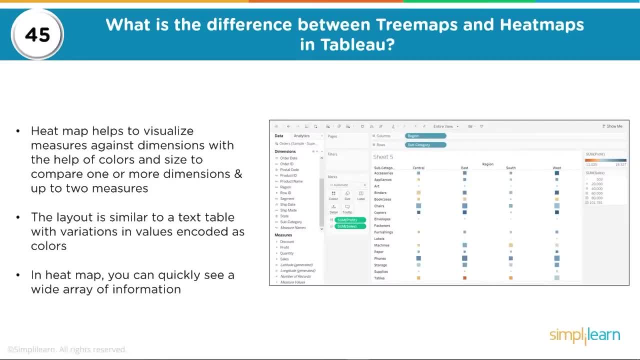 And the size of the little square to denote something else. A lot of times you can even graph this into a three dimensional graph With other data, so it pops out. But again, a heat map is the color and the size Using the sample superstore data set. 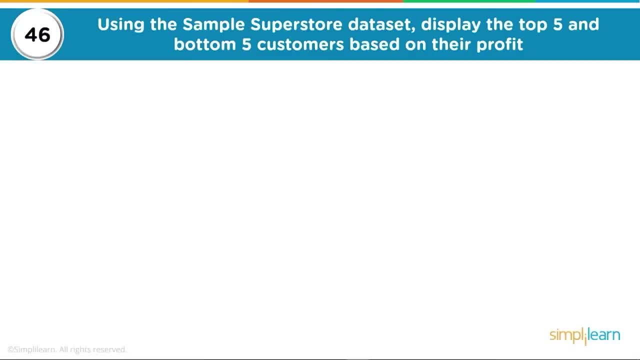 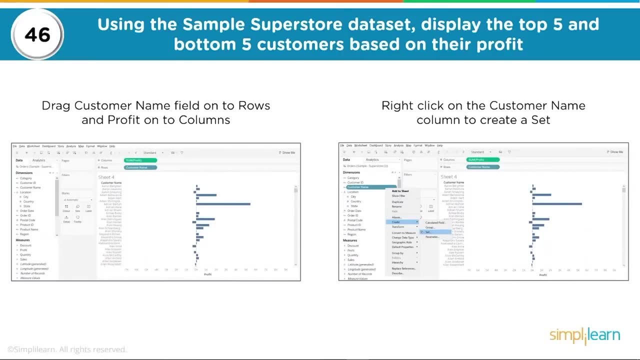 Display the top five and bottom five customers Based on their profit. So you start by dragging the customer name field Onto rows and profit on columns. Right click on the customer name column to create a set. Give a name to the set and select top tab. 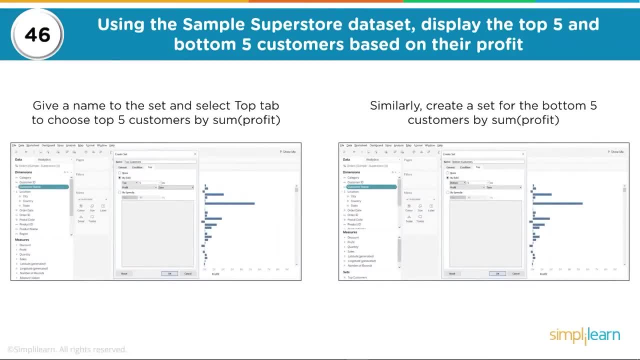 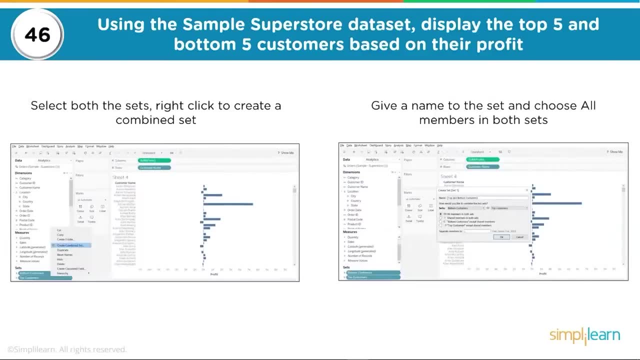 To choose top five customers by some profit. Similarly, create a set for the bottom five customers by some profit. Select both the sets, Right click to create a combined set, Give a name to the set and choose all members in both sets, And then you can drag top and bottom customer sets. 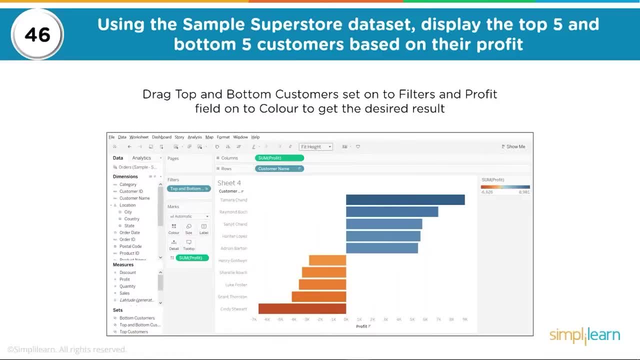 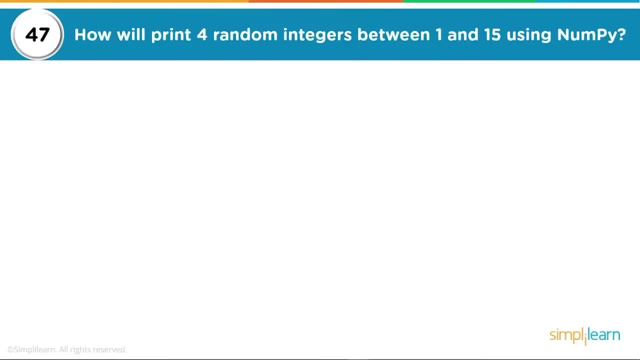 Onto the filters and profit field Onto color to get the desired results. As we get down to the end Of our list, We're going to try to keep you on your toes. We're going to skip back to numpy: How to print four random integers. 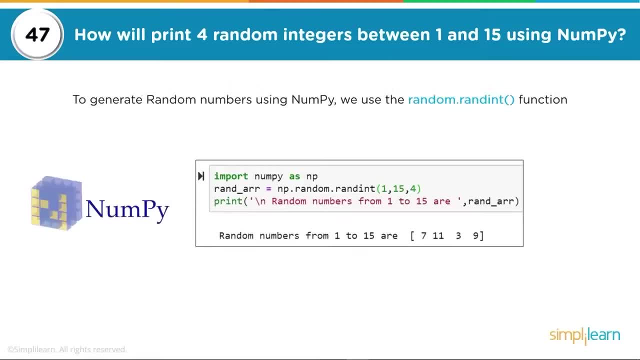 Between one and fifteen using numpy. To generate random numbers using numpy We use the random integer function. You can see here we did the import. Numpy is in p. Random arrangement equals in p dot. random dot. random integer. One through fifteen of four. 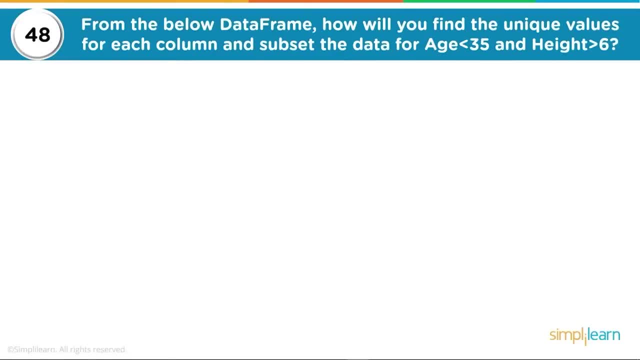 From the below data frame. Going to jump again on you Now, we're into pandas. How will you find the unique values For each column in the subset, The data for age less than thirty five And height greater than six? To find the unique values. 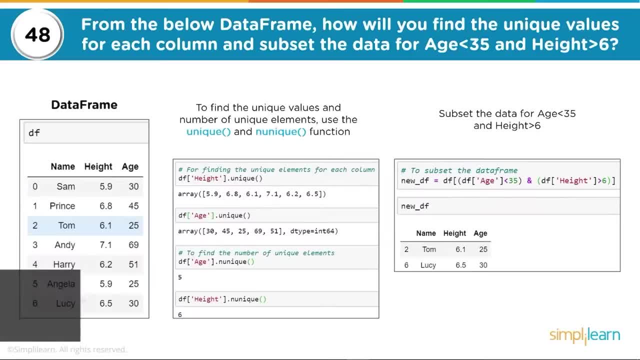 And the number of unique elements. Use the unique and the in unique function. You can see here we just did df heights. We're selecting just the height column And we want to look for the unique. That returns an array Where in unique? 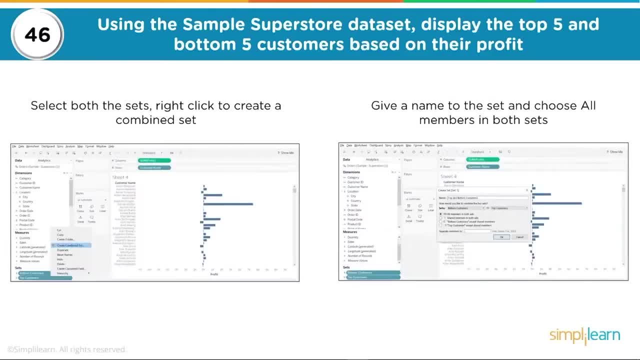 the bottom five customers by some profit. the bottom five customers by some profit. select both the sets. right-click to select both the sets. right-click to select both the sets. right-click to create a combined set. give a name to the. create a combined set. give a name to the. 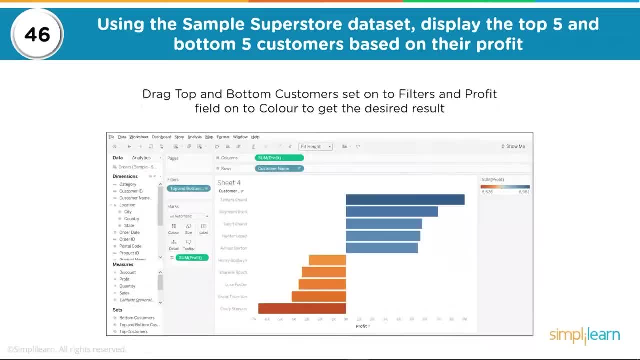 create a combined set, give a name to the set and choose all members in both sets. set and choose all members in both sets. set and choose all members in both sets and then you can drag top and bottom, and then you can drag top and bottom, and then you can drag top and bottom customer sets on to the filters and 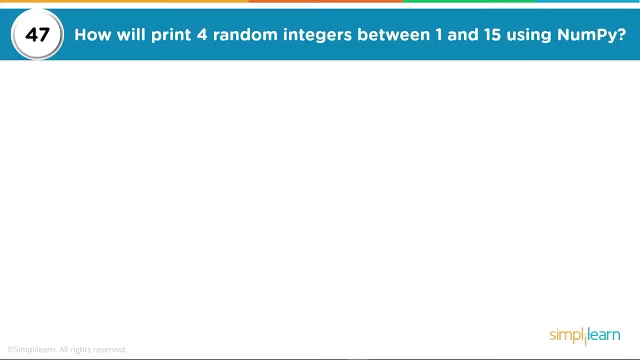 customer sets on to the filters. and customer sets on to the filters and end of our list. we're gonna try to keep you end of our list. we're gonna try to keep you end of our list. we're gonna try to keep you on your toes. we're gonna skip back to. 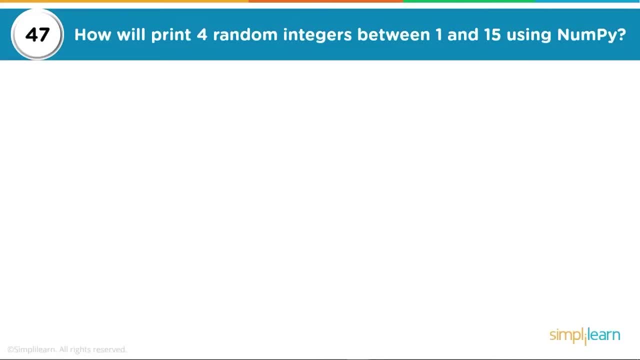 on your toes. we're gonna skip back to on your toes. we're gonna skip back to numpy: how to print four random integers. numpy- how to print four random integers. numpy. how to print four random integers between 1 and 15. using numpy to generate. between 1 and 15. using numpy to generate. 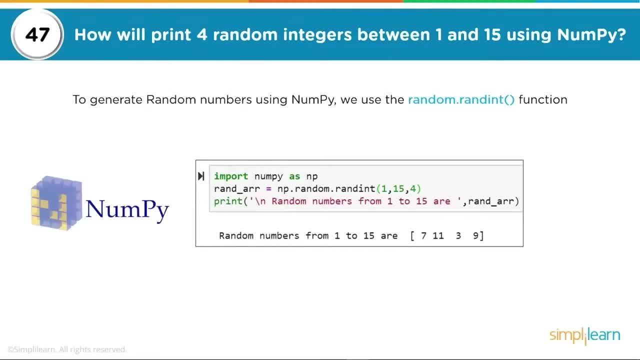 between 1 and 15 using numpy to generate random numbers using numpy. we use the random numbers using numpy. we use the random numbers using numpy. we use the random random integer function. you see random random integer function. you see random random integer function. you see, here we did the import numpy as in P. 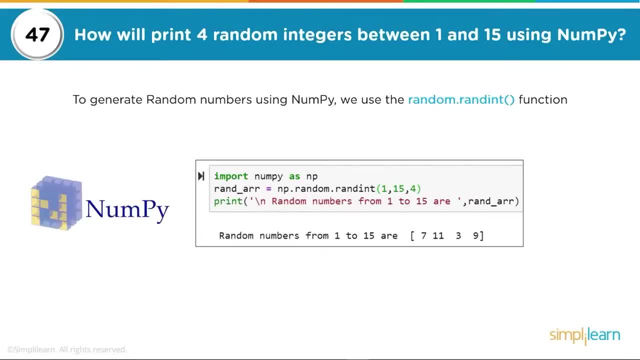 here we did the import numpy as in P. here we did the import numpy as in P. random arrangement equals in P dot. random random arrangement equals in P. dot. random random arrangement equals in P. dot. random dot random integer 1 through 15 of dot. random integer 1 through 15 of. 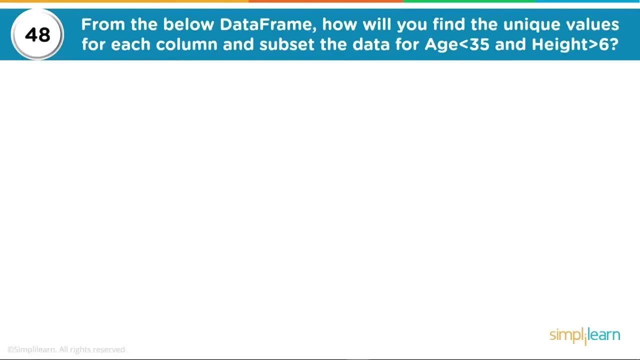 dot random integer 1 through 15 of 4 from the below data frame can jump 4 from the below data frame can jump 4 from the below data frame can jump. again on you now we're into pandas, how. again on you now we're into pandas, how. 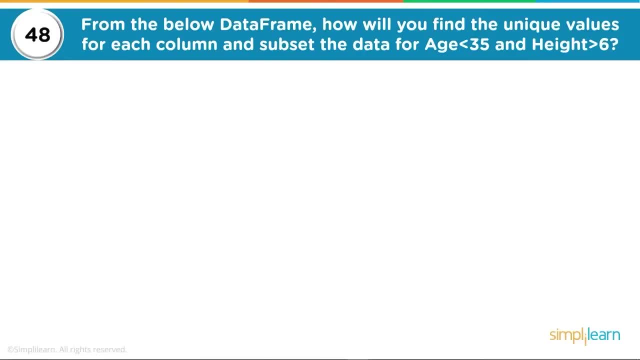 again on you. now we're into pandas. how will you find the unique values for each? will you find the unique values for each? will you find the unique values for each column and subset the data for age less column and subset the data for age less column and subset the data for age less than 35 and height greater than 6 to. 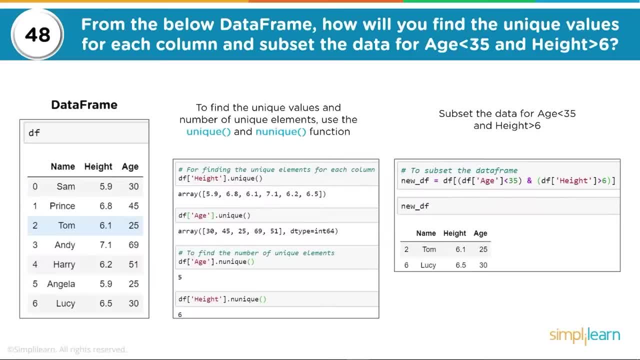 than 35 and height greater than 6 to than 35 and height greater than 6. to find the unique values and the number of. find the unique values and the number of. find the unique values and the number of unique elements. use the unique and the in. 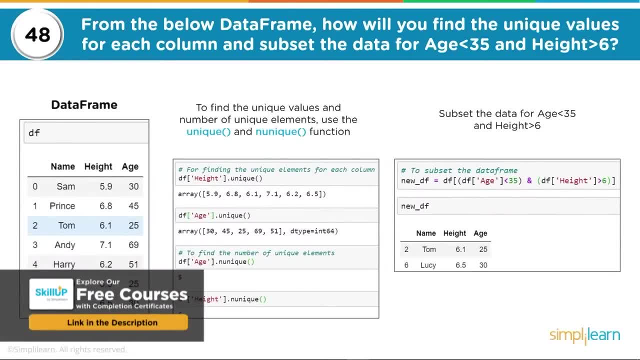 unique elements. use the unique and the in unique elements. use the unique and the in unique function. you can see, here we just unique function. you can see, here we just unique function. you can see, here we just did DF heights, we're selecting just the. did DF heights, we're selecting just the. 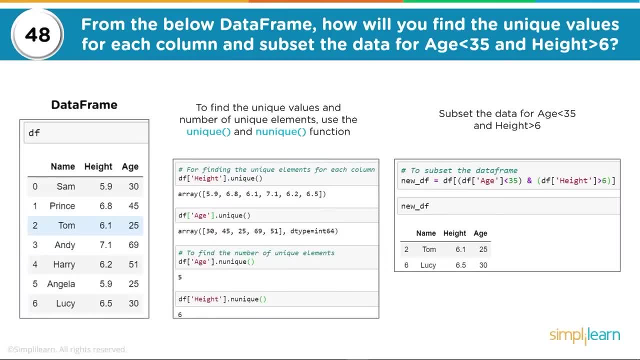 did DF heights. we're selecting just the height column and we want to look for height column. and we want to look for height column and we want to look for the unique that returns an array. where in the unique that returns an array. where in the unique that returns an array. where in unique. if we do that on the height or 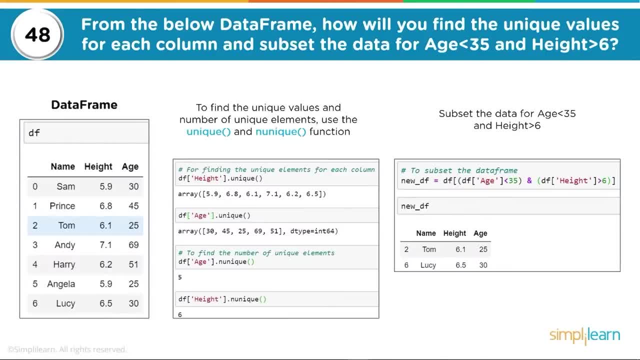 unique, if we do that on the height, or unique, if we do that on the height or the age, will return just the number of the age, will return just the number of the age will return, just the number of unique values, and then we can do a- unique values and then we can do a. 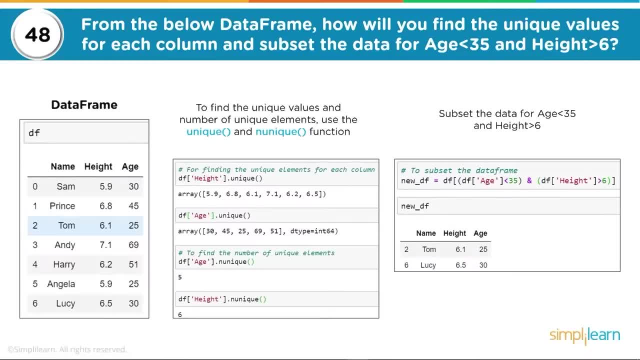 unique values and then we can do a subset the data for ages less than 35 and subset the data for ages less than 35. and subset the data for ages less than 35 and height greater than 6. so, if you look, height greater than 6. so if you look, 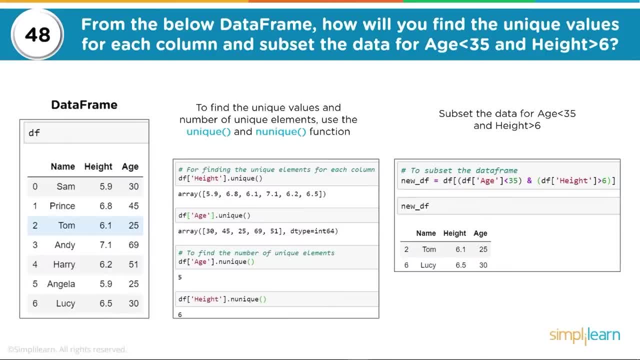 If we do that on the height Or the age, Return just the number of unique values And then we can do a subset: the data For ages less than thirty five And height greater than six. So if you look over here, We have a new df. 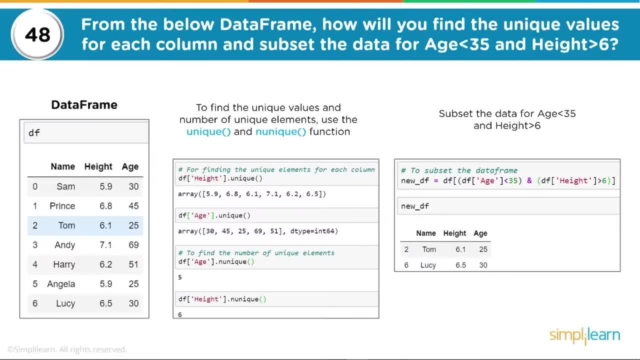 Remember this is going to be taking slices Of our original data frame. It doesn't actually change the data frame. So our new df equals The data frame or df, The data frame where age is less than thirty five And the height is greater than six. 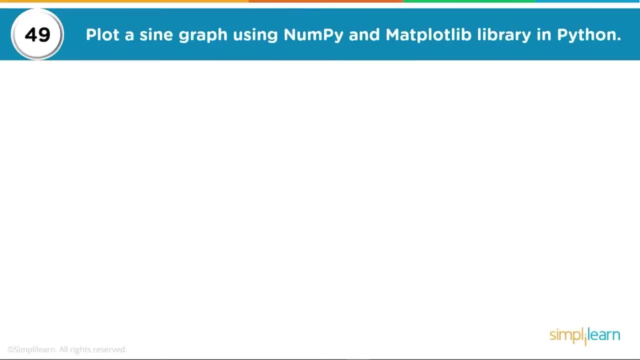 And in case you're not using tab blue, Which has a lot of its own Different mapping programs in there, Make sure you understand how to use the basics Of matplot library. Plot a sign graph using numpy And matplot library in python. 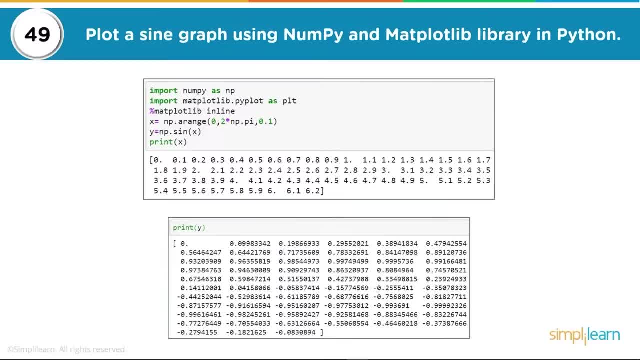 And the way we did this Is: we went ahead and generated an x. We know our y equals np, Sine of x. If you print out x, You'll see a whole value here. Our matplot library, piplot As plt. 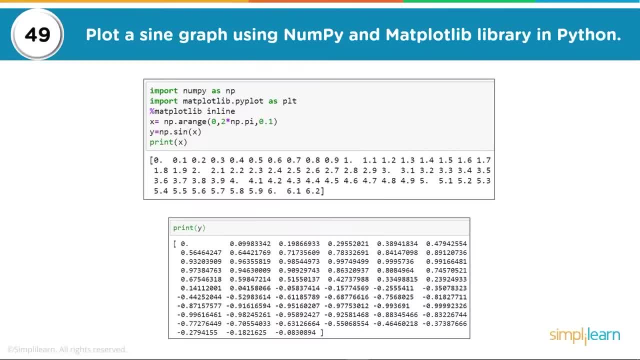 If you are working in jupiter notebook Make sure you understand The matplot library inline, That little percentage sign Matplot library inline That prints it on the page in the jupiter notebook. The newer version of jupiter notebook Or jupiter labs automatically does that for you. 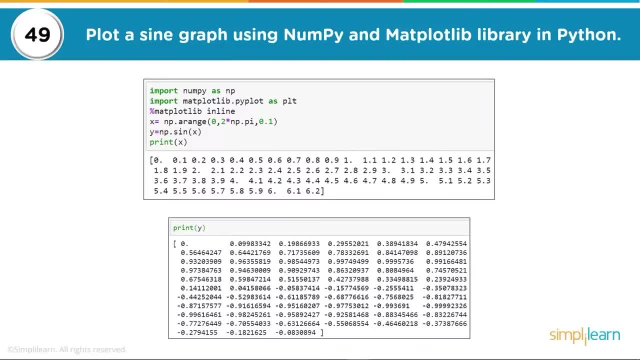 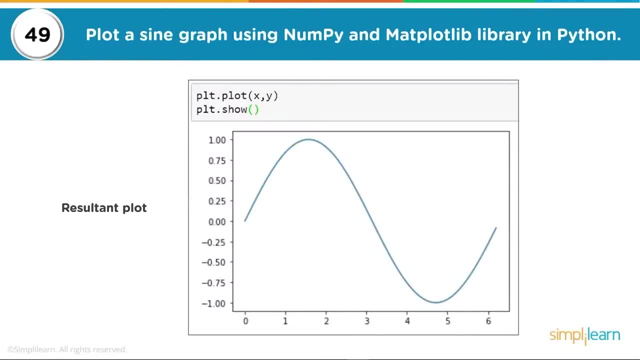 But I usually put it in there, Just in case I end up on an older version. If you print y, You can see here we have our different y values And our different x values. You simply put in pltplot xy And that's it. 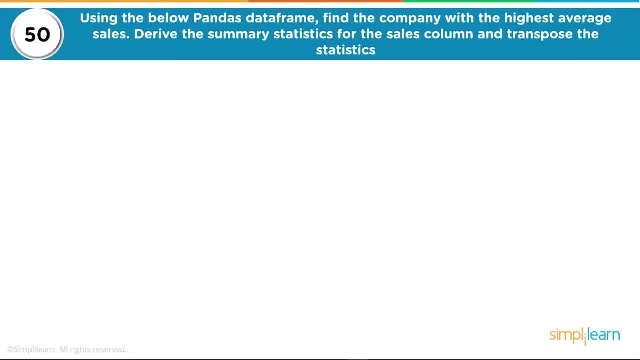 And before we go, Let's get one more in. We're going to do a pandas Using the below pandas data frame. Find the company with the highest average cells, Derive the summary statistics for the cells column And transpose these statistics. 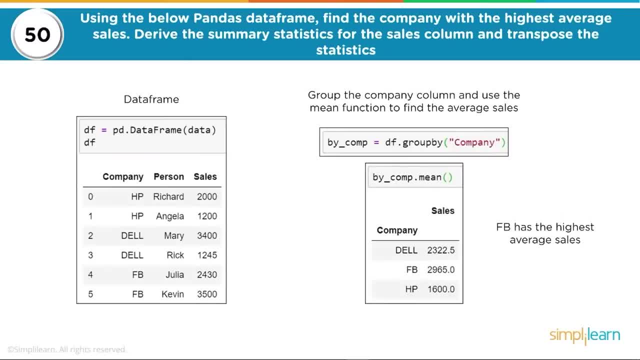 That's a mouthful And, just like any of these computer problems, Break it apart. So first of all We're looking for the highest average cells. So group the company column And use the mean function To find the average cells. 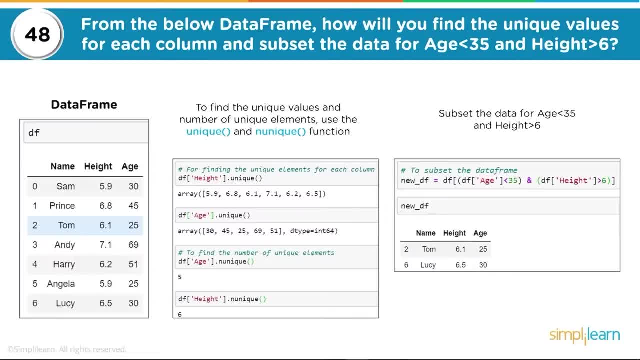 height greater than 6. so if you look over here, we have a new DF. remember this. over here, we have a new DF, remember this. over here, we have a new DF, remember this. is going to be taking slices of our. is going to be taking slices of our. 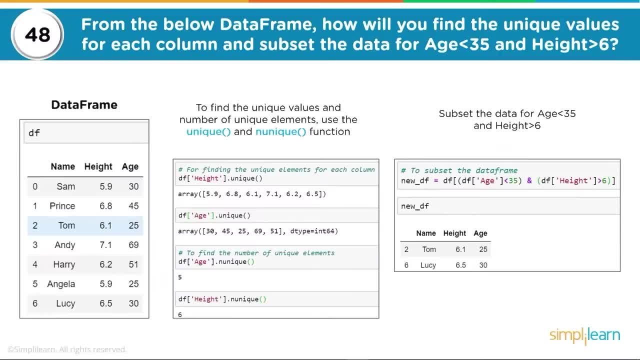 is going to be taking slices of our original data frame. it doesn't actually original data frame. it doesn't actually original data frame. it doesn't actually change the data frame. so our new DF change the data frame. so our new DF change the data frame. so our new DF equals the data frame or DF the data. 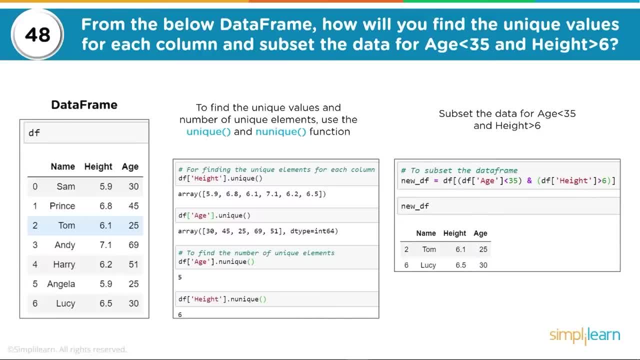 equals the data frame or DF. the data frame or DF. the data frame or DF. the data frame where age is less than 35 and the frame where age is less than 35 and the frame where age is less than 35 and the height is greater than 6. 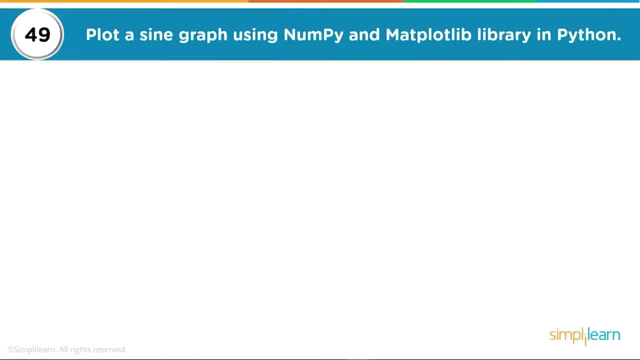 height is greater than 6. height is greater than 6, and in case you're not using tab blue, and in case you're not using tab blue, and in case you're not using tab blue, which has a lot of its own different, which has a lot of its own different. 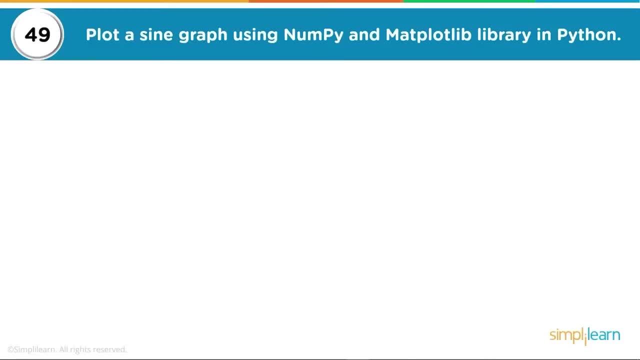 which has a lot of its own different mapping programs in there. make sure you mapping programs in there. make sure you mapping programs in there. make sure you understand how to use the basics of mat. understand how to use the basics of mat. understand how to use the basics of mat. plot library. plot a sign graph using. 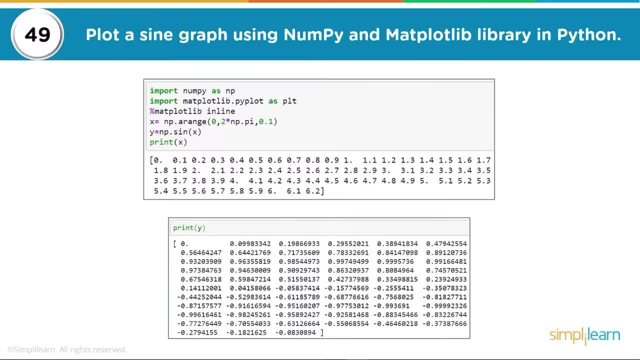 plot library. plot a sign graph using plot library. plot a sign graph using numpy and mat plot library and Python: numpy and mat plot library and Python, numpy and mat plot library and Python. and the way we did this is we went ahead, and the way we did this is we went ahead. 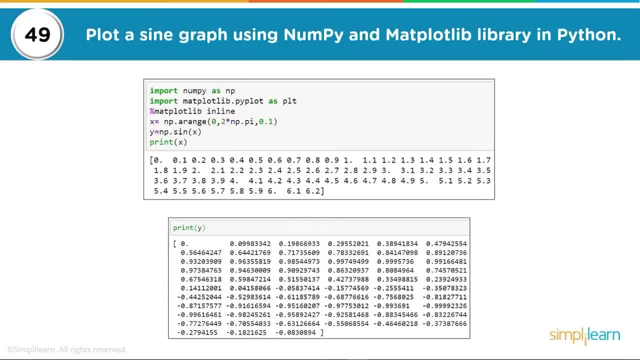 and the way we did this is: we went ahead and generate an X. we know our Y equals and generate an X. we know our Y equals and generate an X. we know our Y equals NP sine of X. if you print out X, you'll NP sine of X. if you print out X, you'll. 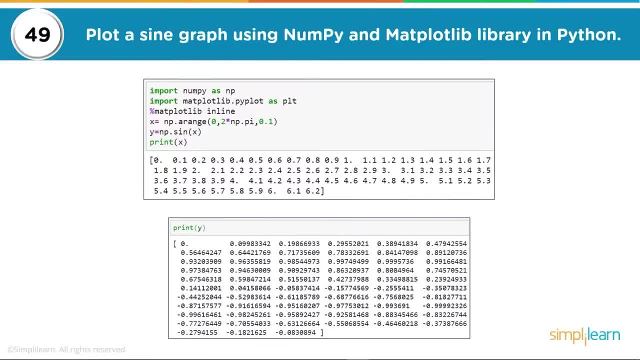 NP sine of X. if you print out X, you'll see a whole value here, our mat plot. see a whole value here, our mat plot. see a whole value here, our mat plot. library pi plot as PLT if you are. library pi plot as PLT if you are. 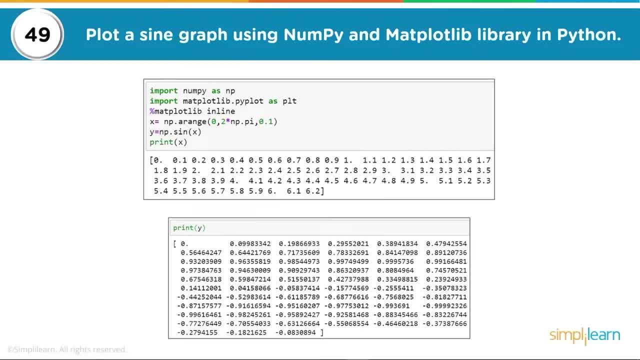 library pi plot as PLT. if you are working in Jupiter notebook, make sure, working in Jupiter notebook, make sure, working in Jupiter notebook, make sure you understand the mat plot library in you understand the mat plot library in. you understand the mat plot library in line that little percentage sign mat. 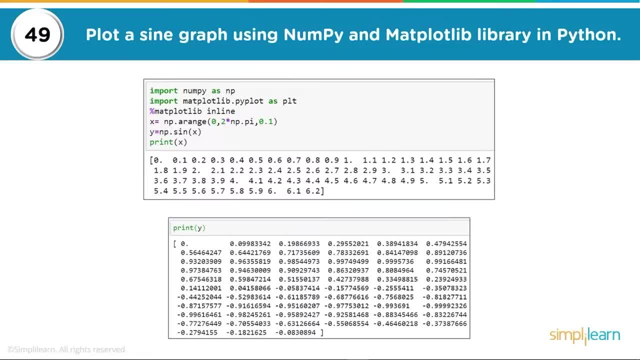 line that little percentage sign mat line. that little percentage sign mat. plot library in line. that prints it on plot library in line. that prints it on plot library in line. that prints it on the page in the Jupiter notebook. the the page in the Jupiter notebook. the the page in the Jupiter notebook. the newer version of Jupiter notebook. or. 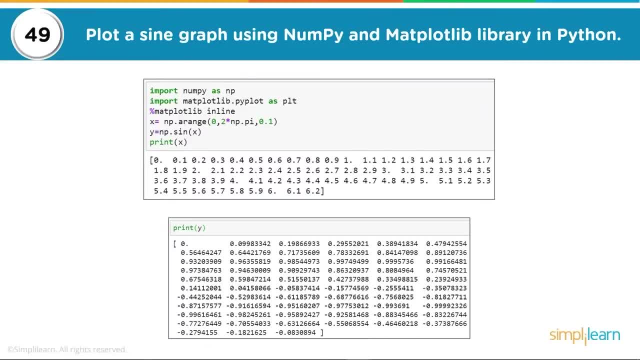 newer version of Jupiter notebook or newer version of Jupiter notebook or Jupiter labs. automatically does that for Jupiter labs. automatically does that for Jupiter labs. automatically does that for you. but I usually put it in there, just you. but I usually put it in there, just you. but I usually put it in there just in case I end up on an older version if in case I end up on an older version, if in case I end up on an older version, if you print why you can see here we have you print. why you can see here we have you print. why you can see here we have our different Y values and our different. 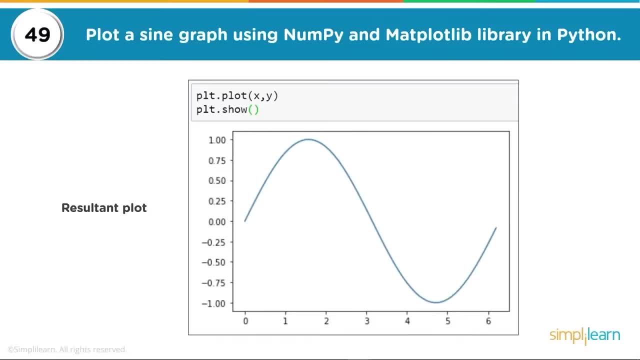 our different Y values and our different. our different Y values and our different X values. you simply put in PLT dot plot X values. you simply put in PLT dot plot X values. you simply put in PLT dot plot X, Y and do a plot show. and before we go, 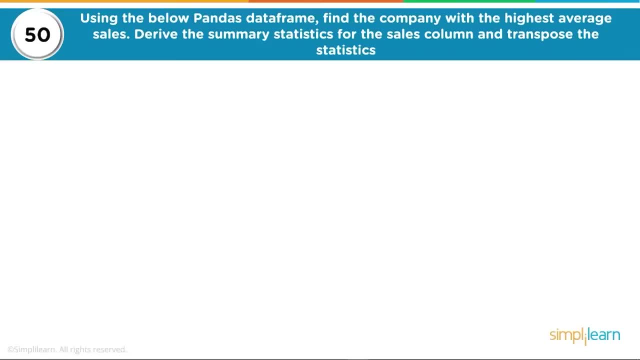 X, Y and do a plot show. and before we go, X, Y and do a plot show, and before we go, let's get one more in. we're going to do, let's get one more in. we're going to do, let's get one more in. we're going to do a pandas using the below pandas data: 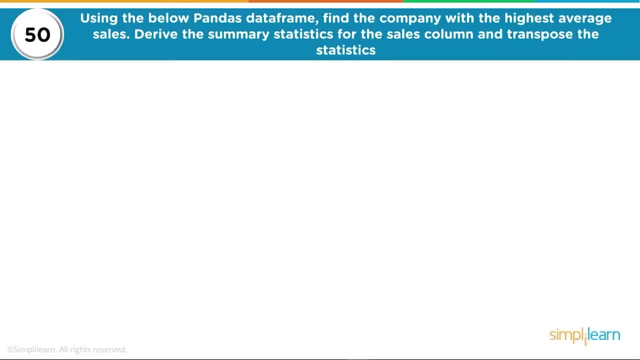 a pandas using the below pandas data: a pandas using the below pandas data frame. find the company with the highest frame. find the company with the highest frame. find the company with the highest average cells. derive the summary average cells. derive the summary average cells. derive the summary statistics for the cells column and. 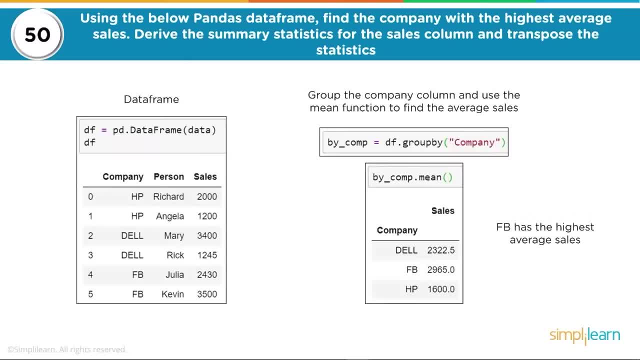 statistics for the cells column and statistics for the cells column and transpose these statistics. that's a. transpose these statistics. that's a transpose these statistics. that's a mouthful and just like any of these mouthful and just like any of these mouthful and just like any of these computer problems, break it apart. so, 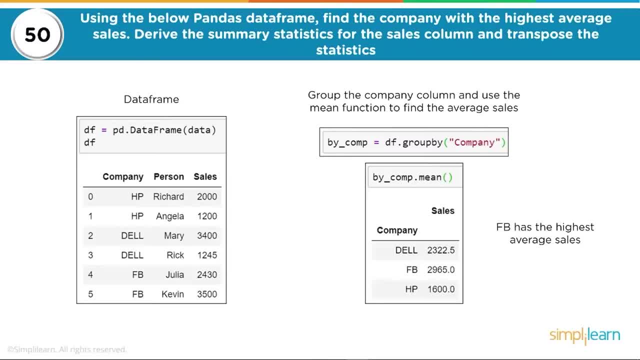 computer problems break it apart. so computer problems break it apart. so first of all we're looking for the first of all. we're looking for the first of all. we're looking for the highest average cells, so group the highest average cells, so group the highest average cells. so group the company column and use the mean function. 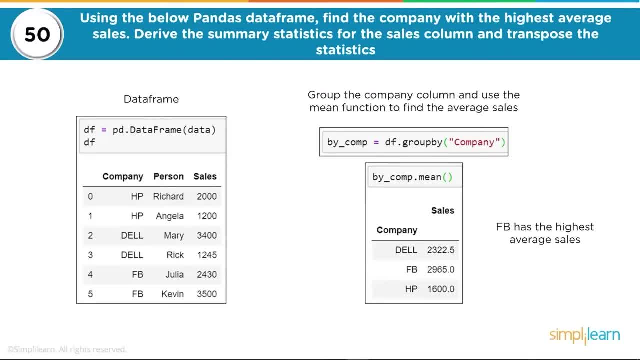 company column and use the mean function, company column and use the mean function to find the average cells. and you see, to find the average cells. and you see to find the average cells. and you see, here by company equals, DF group by. here by company equals, DF group, by. 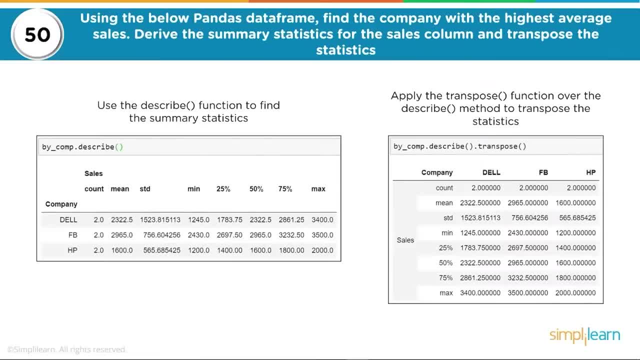 here by company equals DF group by company. once we've done that using the company, once we've done that using the company, once we've done that using the describe function, we can now go ahead describe function. we can now go ahead describe function. we can now go ahead and look at the summary of statistics on 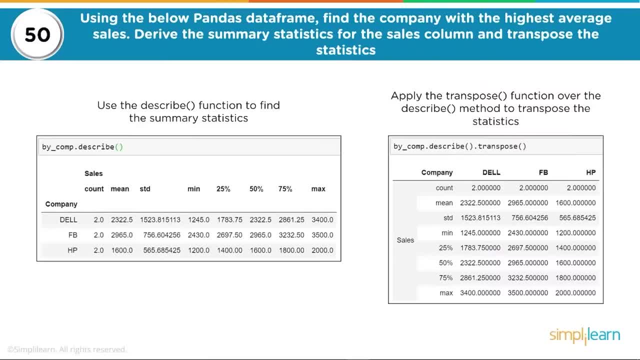 and look at the summary of statistics on: and look at the summary of statistics on here. use the describe function to find here. use the describe function to find here. use the describe function to find the summary. so by company. those are the summary. so by company. those are. 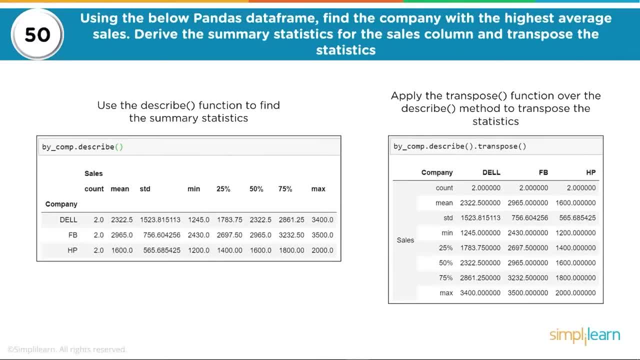 the summary. so by company, those are groups. we're just going to describe them groups. we're just going to describe them groups. we're just going to describe them and you could actually bundle those and you could actually bundle those, and you could actually bundle those together if you wanted, and just do them. 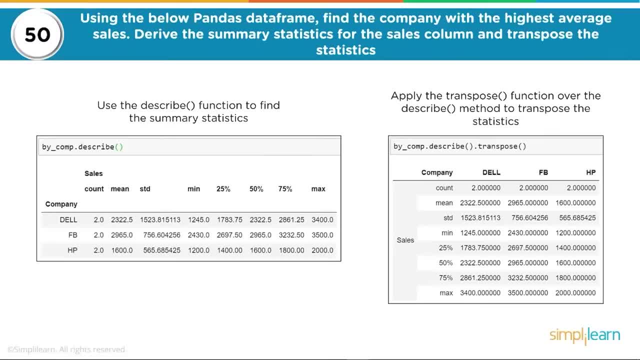 together if you wanted, and just do them together if you wanted and just do them all in one line. so here we go by: company all in one line. so here we go by company all in one line. so here we go by company dot describe. you can see we have a nice. 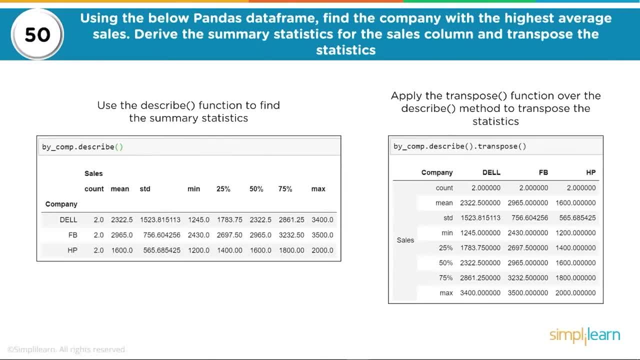 dot describe. you can see we have a nice dot describe. you can see we have a nice breakout always good to remember whether breakout always good to remember, whether breakout always good to remember whether you're using any of the packages where you're using any of the packages where 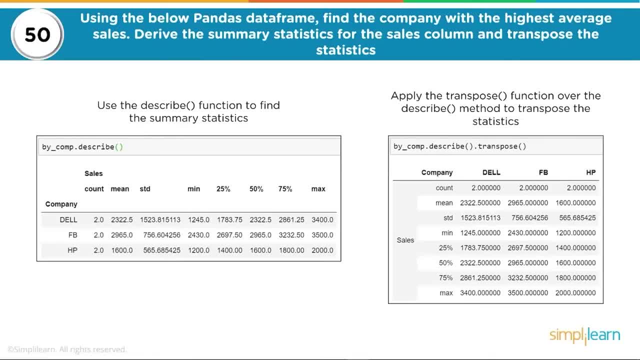 you're using any of the packages where there's tab blue or pandas in Python, or there's tab blue or pandas in Python, or there's tab blue or pandas in Python or even are, or some other package being even are, or some other package being even are, or some other package being able to quick look and describe your. 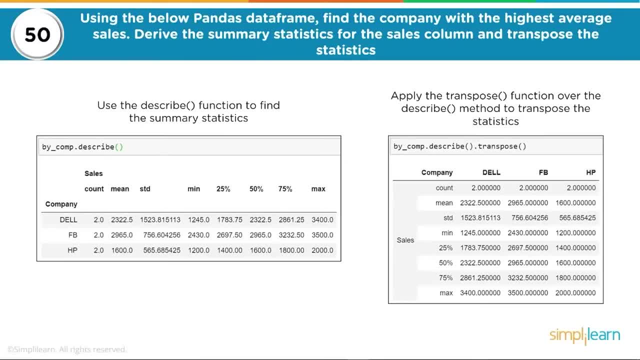 able to quick look and describe. your able to quick look and describe your data is very important. and then we go: data is very important and then we go: data is very important and then we go ahead. just do a basic apply, a transpose ahead. just do a basic apply, a transpose. 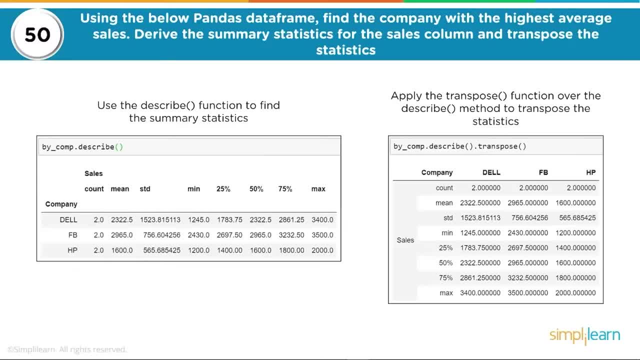 ahead. just do a basic, apply a transpose function over the describe method. to function over the describe method to function over the describe method. to transpose the statistics. all we've done: transpose the statistics. all we've done, transpose the statistics. all we've done here is flip the index with the column.